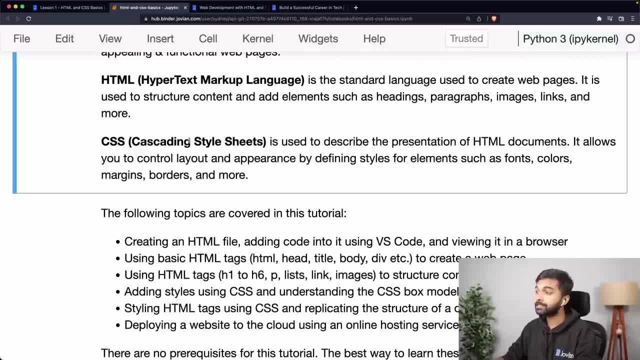 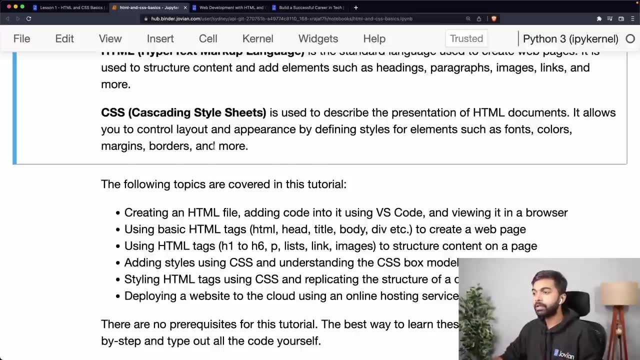 cascading style sheets, or CSS, is used to describe the presentation of HTML documents. It allows you to control the layout and the appearance by defining styles or elements, and you can configure things like fonts, colors, margins, borders, etc. So today we are going to look at the very basics of HTML and CSS. We are going to start by creating 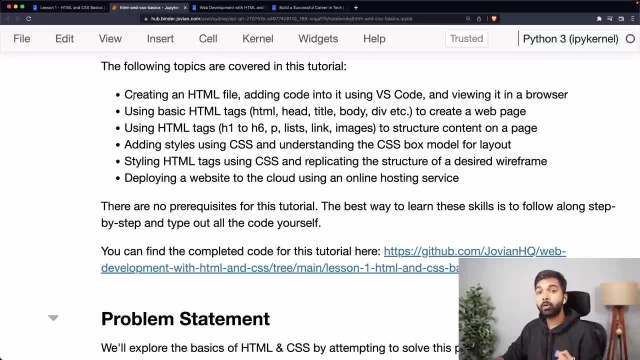 an HTML file, adding code into it using the VS code editor, viewing it in a browser. We're going to then use some basic HTML tags to create a web page. Then we're also going to use some more HTML tags to structure content. We're also going to use some more HTML tags to structure content. 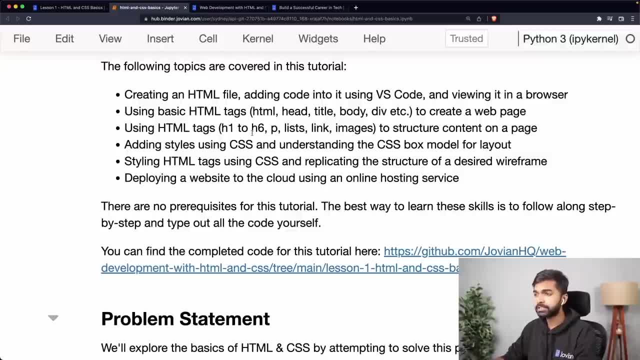 content on a page, things like headings, lists, paragraphs, etc. Then we're going to add styles using CSS and understand the CSS box model for layout. that is the core, foundational concept in CSS. And then we're going to style these HTML tags. 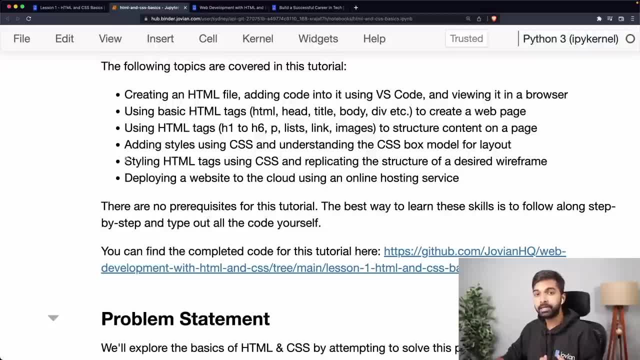 using CSS to replicate the structure of a desired web page. So we look at a problem statement and we'll try to replicate the web page that we have in mind using HTML and CSS. And finally, if time permits, we are also going to try and deploy. 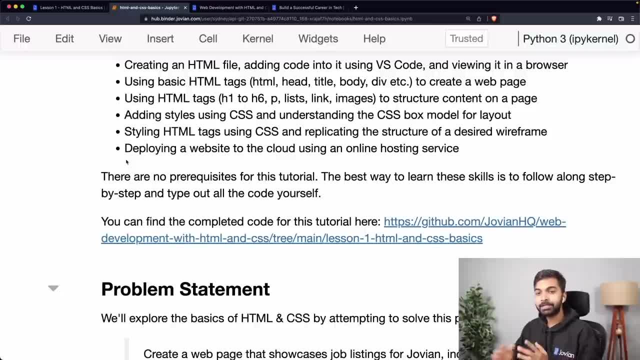 that website to the cloud using an online hosting service. So in just about two and a half hours from now, you will be in a position where you will have deployed your first website to the cloud. So isn't that exciting: the first, very first. 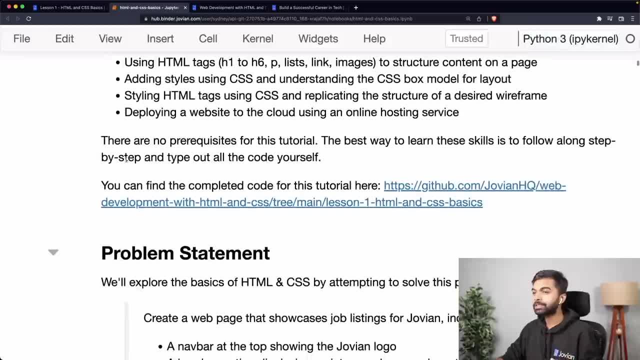 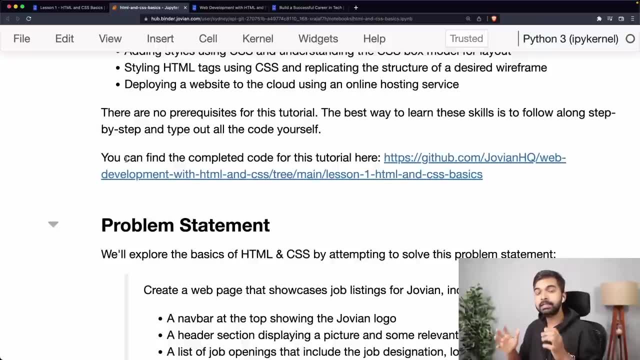 lesson. you will be deploying your own website, And there are no prerequisites for this tutorial. the best way for you to learn these skills is to follow along. As you're watching the lesson, pause it at various places, follow along and then you will be able to deploy your website to the 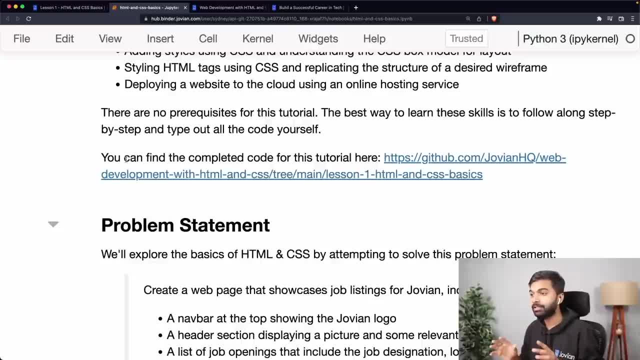 cloud. So as you're watching the lesson, pause it at various places, follow along, type out all the code yourself. don't even copy paste, just type everything out And then experiment with it using the exercises that are present in the lesson. Now you 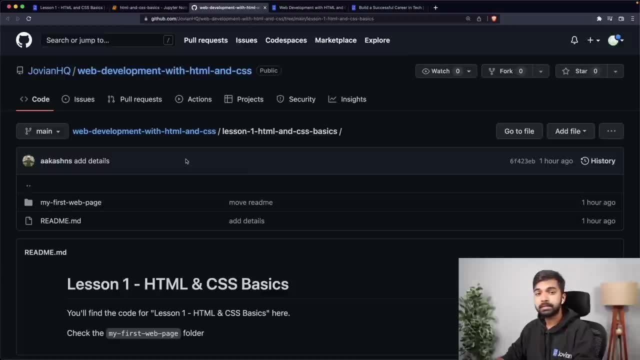 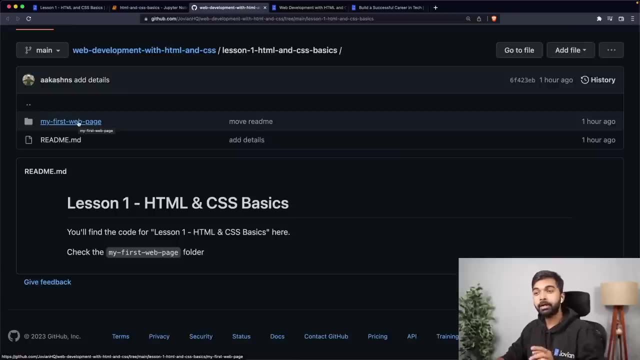 can find the completed code for this tutorial here in this GitHub repository. Specifically, you can open up this folder- my first web page- and you will find all the code that we are covering today in this folder. So we will explore the basics of 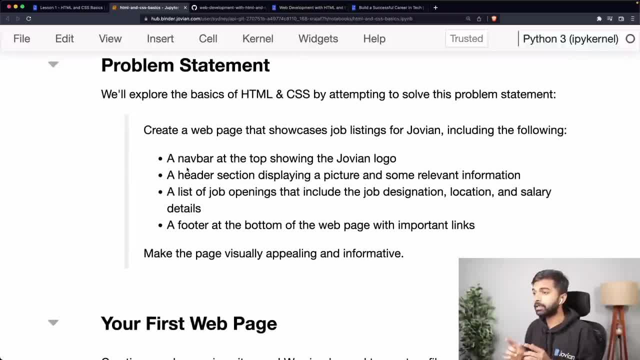 HTML and CSS. by attempting to solve this problem statement, We will create a web page that showcases job listings for Jovian. At Jovian, we have a growing team. we have a growing user base. we're adding new programs, So we have certain jobs for which we 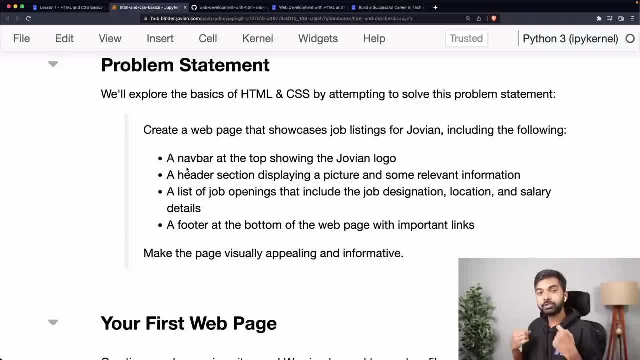 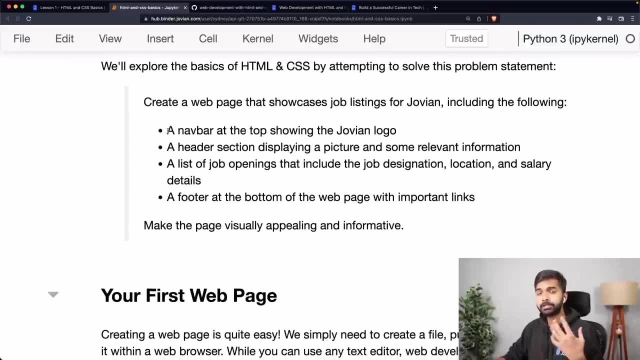 want to hire, but we don't have a jobs page yet. So we're going to try and create a jobs page for Jovian And on this jobs page we're going to show a few things. we're going to require our job space to have a few things. One is a navbar at the 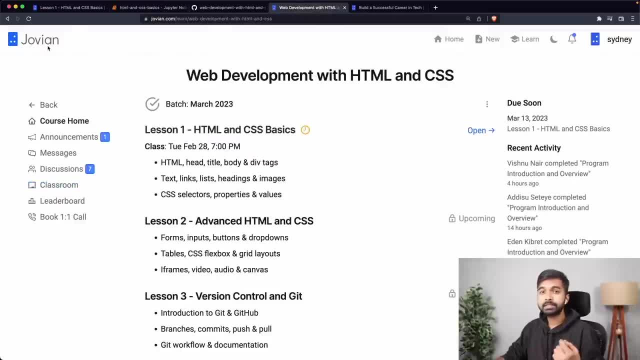 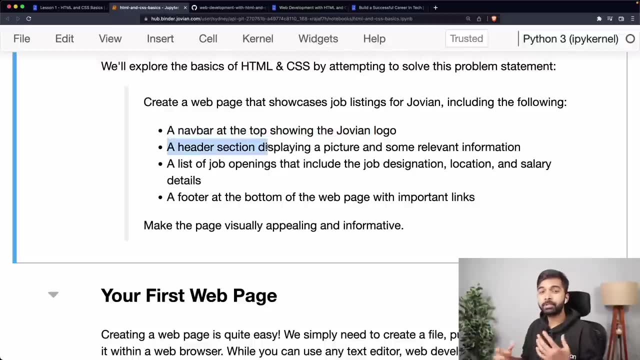 top showing the Jovian logo. So something like this. this is called a navigation bar or a navbar. Then we may want a header section displaying a picture and some relevant information about Jovian. So anybody who comes to our jobs page should learn a little bit about the company. 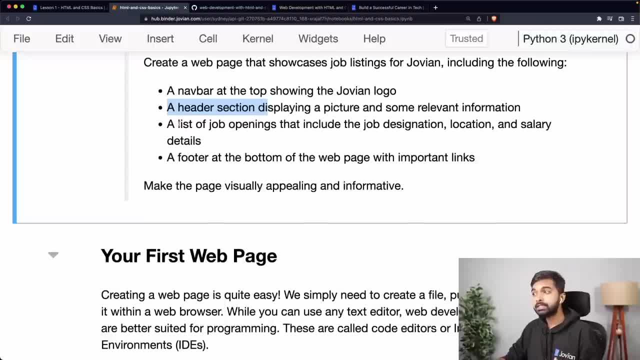 itself. So we'll have that, Then maybe a list of job openings that include the job designation, location and maybe salary details. we'll see what we can put in there- And maybe also a link to apply for the job And then a footer at the. 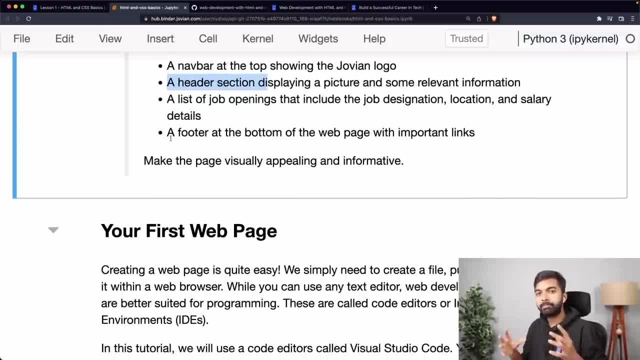 bottom of the web page with some important links. So generally at the bottom of any web page in a website you might include, you might have a bunch of links to other web pages on the same website or elsewhere. So we are going to try and build all of this today in the next couple. 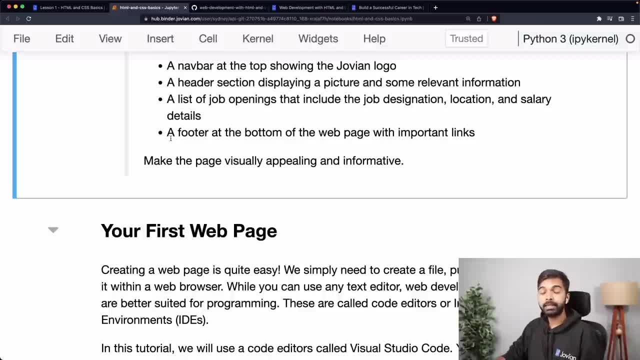 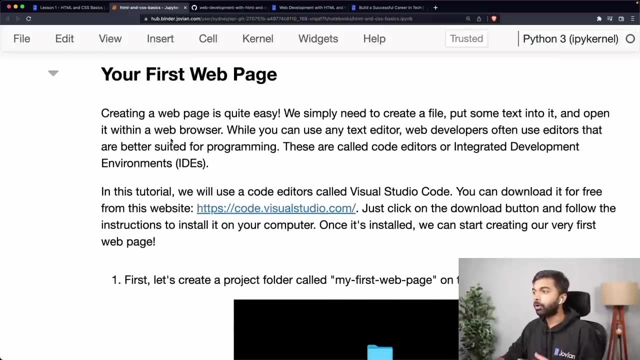 of hours, And we will also attempt to make the page visually appealing and informative. Let's see how far we can get. This is a fairly ambitious problem statement. while we are also learning the basics of HTML and CSS Now, creating your first web page is actually quite easy. All you need to do is simply 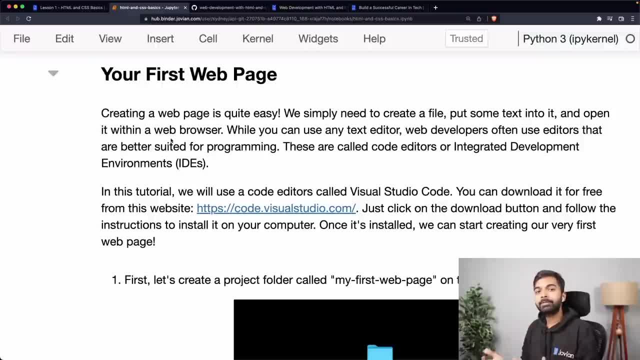 create a file, put some text into it and then open that file browser. And while you can use any text editor to create the file and put some text into it, Web developers often use editors that are better suited for programming because they have certain features that will help you write code in various 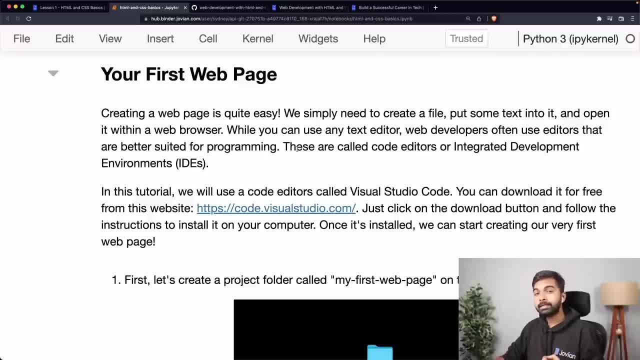 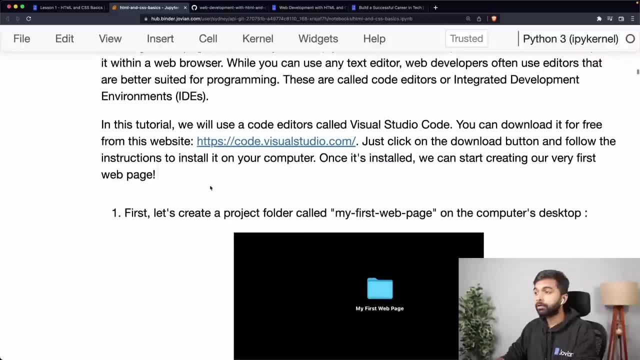 programming languages easily, And these are called code editors or sometimes also called integrated development environments. Okay so, in this tutorial for today, we are going to use a code editor called Visual Studio Code. Now you can download it for free. It is. 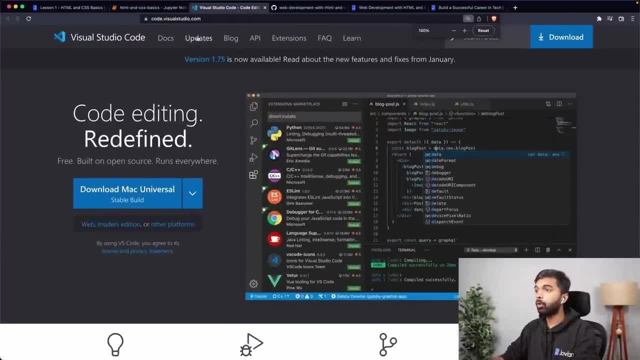 a free and open source tool, So you can download it by going to codevisualstudiocom. All the links are present in the lesson resources and the lesson notebook. Now, based on which operating system you're working on, you will have to download it. 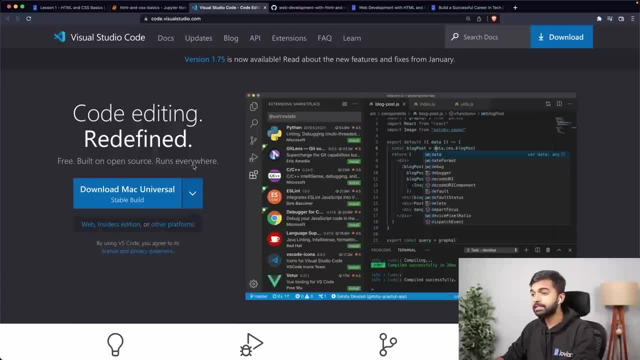 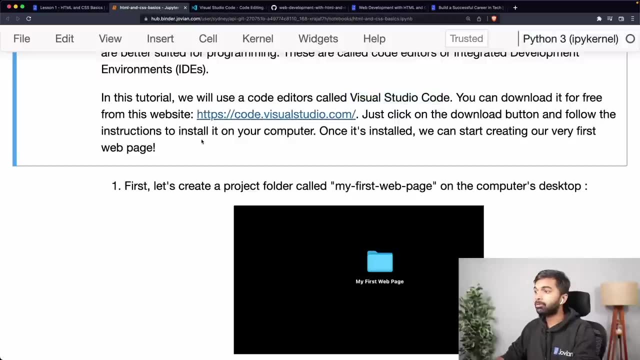 for that operating system. you can see that it is available for all major operating systems And it is developed by Microsoft, So it also has great Windows support And you should download it. And once it is downloaded it just double click the installer and follow the instructions to. 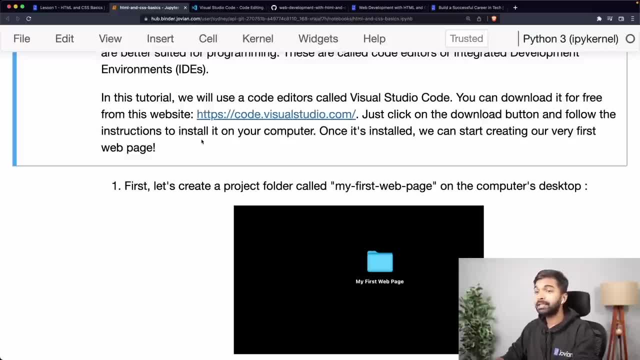 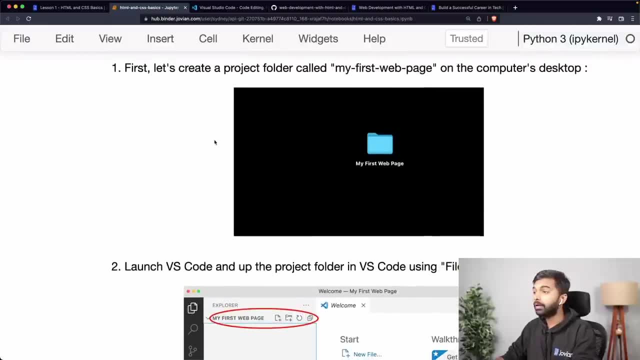 install it on your computer And, once it's installed, we can then start creating our very first web page. Okay, so let's get into it Now. the first thing we need to do is create a project folder. Typically, whenever you're working on a project, it's a. 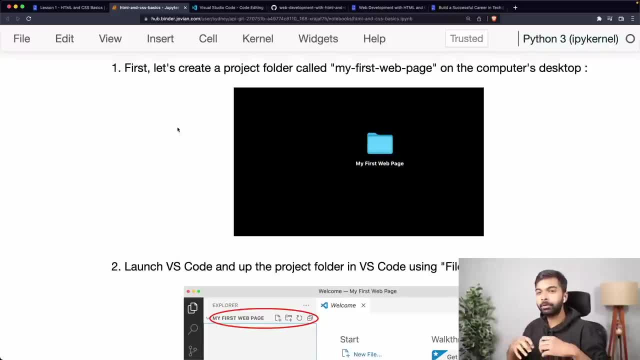 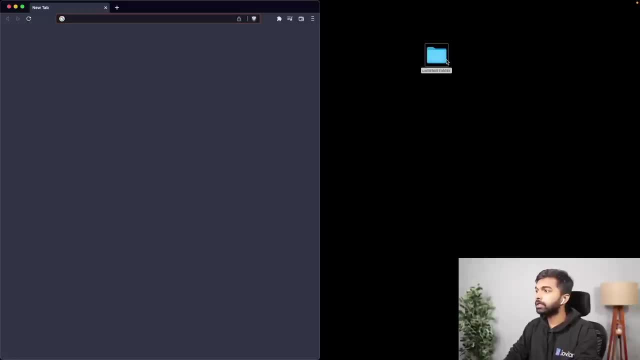 good idea to create a folder. we're going to put all the files so that you don't pull out your desktop or your downloads folder. So let me go in here and let me create a new folder. I'm going to call this folder. 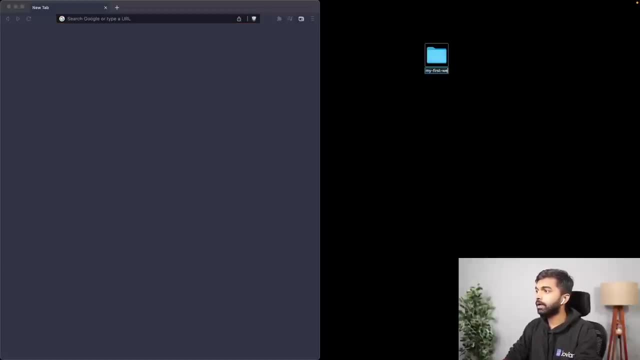 Let's see, I'm going to call this folder my first web page. Okay, I've just used hyphens here. my first web page. If you can't see, let me just zoom in here a little bit. Yeah, so you should be able to see it. now, my first web page. 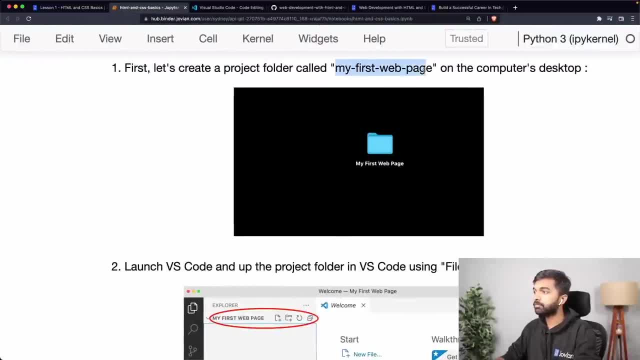 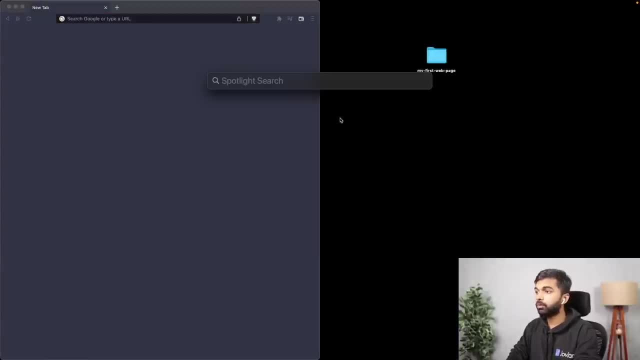 Alright, so I've just used hyphens here. my first web page. that is the name of the folder, And now we want to open up this folder in VS code. So let us first open Visual Studio Code or VS code. Let me just type Visual Studio Code here and open up. 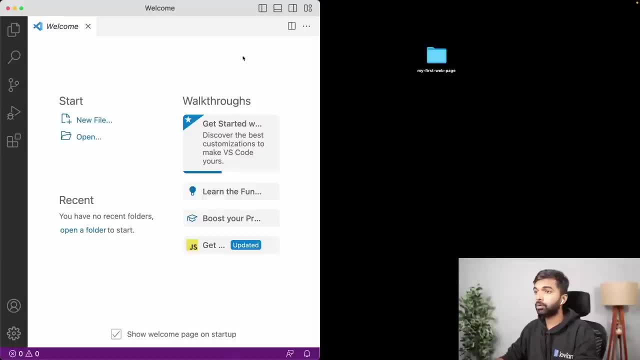 Visual Studio Code. Okay, so now, now I've opened up Visual Studio Code, This is what its user interface looks like. You might also see something like this. you might see a sidebar here as well. So that depends. you can hide or show the sidebar you. 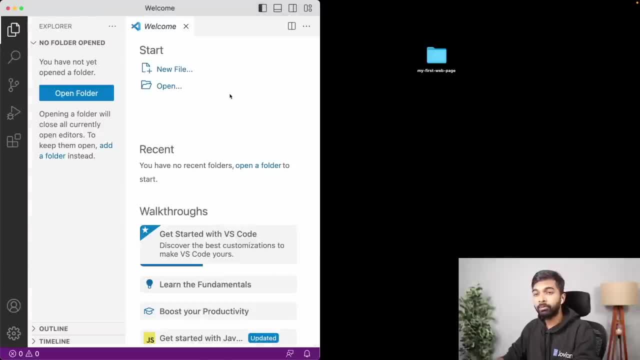 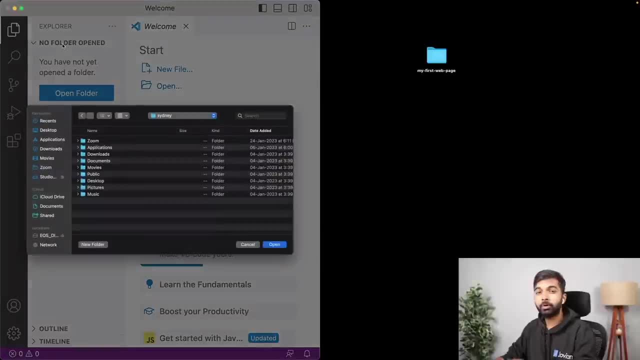 have options to show this over here. Now, what we want to do in Visual Studio Code is open up this folder. Okay, so you want to say file open folder. we're going to the file menu, select open folder, And I'm going to come into my desktop and select this folder. 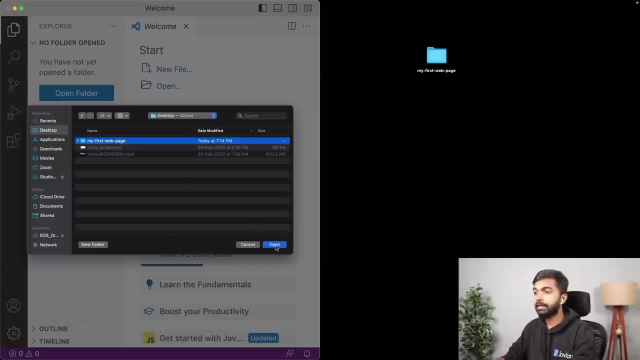 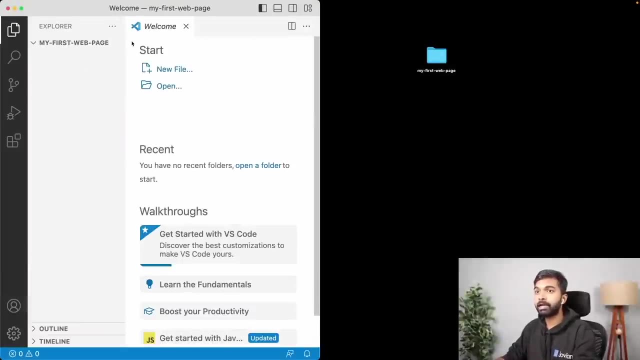 my first web page. don't double click on it, just select it and then click Open. Okay, So now you will immediately see that you will see the folder name here in the sidebar- my first web page. I hope you can see it. And then you'll see this. 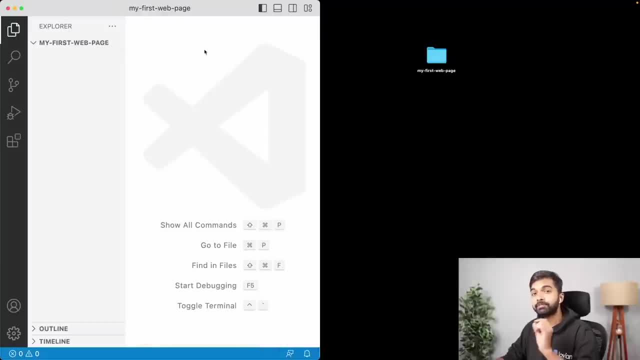 welcome screen. I'm going to close this welcome screen, But now this folder is open in VS code. So VS code is showing us this folder And what I can do is I can now create a file within this folder directly from VS code. 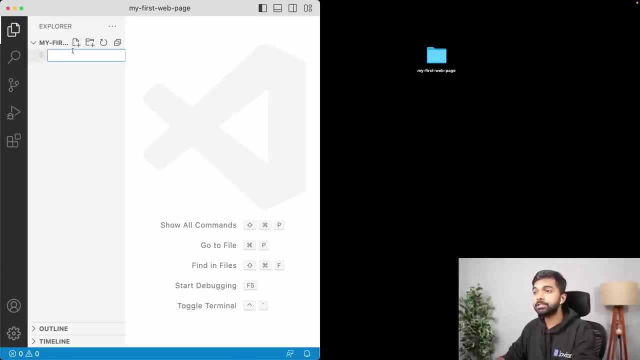 So if I just go here, I should see a new button And in this new button I can, using this new button, I can create a new file. I'm going to create a file called a web page, html, So any web. 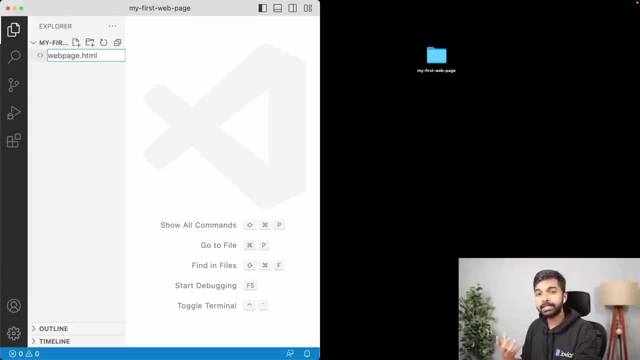 page has the dot html extension, just like images have a dot jpg extension or Excel files dot xls extension, So web pages have the dot html extension. Okay, now I've created this file called web page dot html And I can verify that this file is actually. 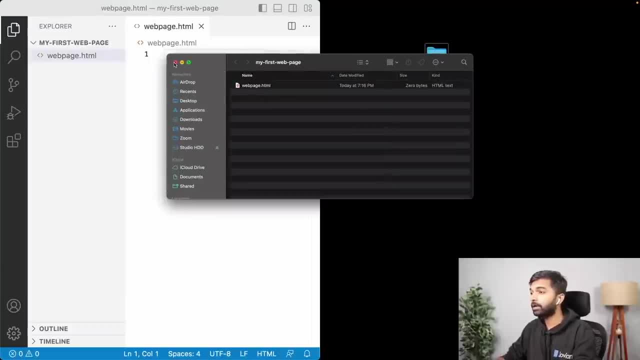 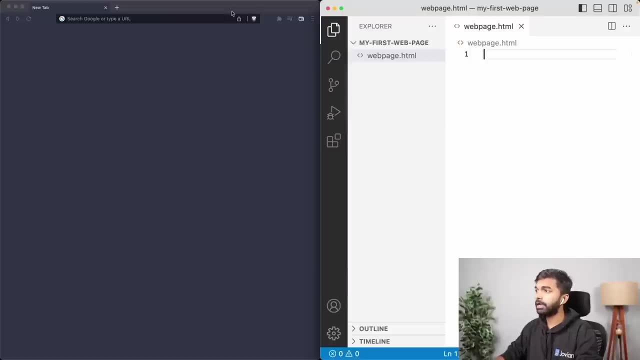 present here: web page dot html. see that when I open that window, when I open that folder, I can see that the file, web page or HTML has been created. Okay, let me just get this on to the right Now, once I've created this. 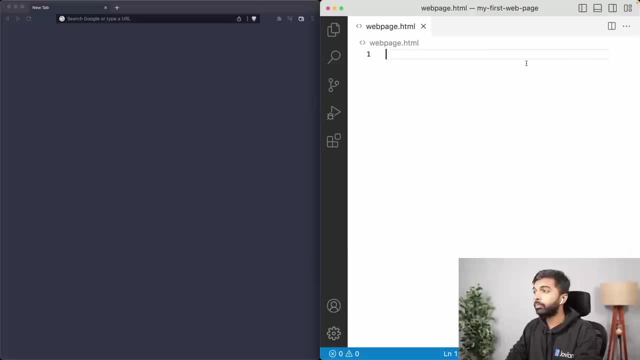 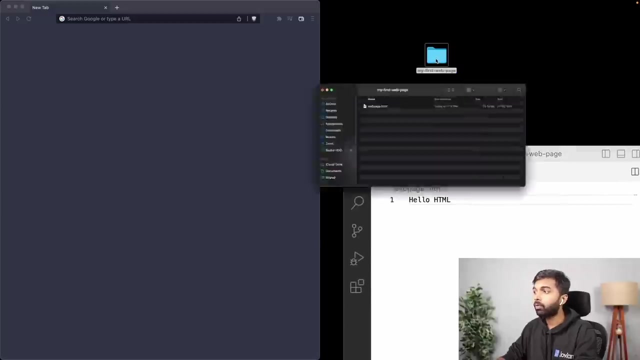 file, web page or HTML, and let me close the sidebar. I'm going to put some text into it, So let me just say Hello HTML, Alright. so I've just written the words Hello HTML into web page or HTML. Alright. now here's what I'm going to do. I am going to now open this. 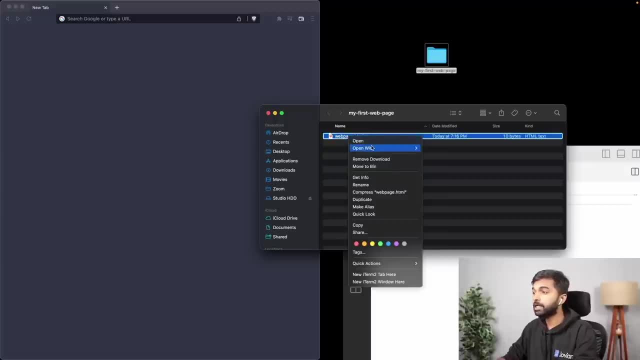 file, web page or HTML in the browser. So I'm going to say open with and I'm going to select the browser that I'm using. Or sometimes you can also just double click and it will automatically open in Google Chrome. But just to be safe, I'm opening it with brave browser. that's the browser. 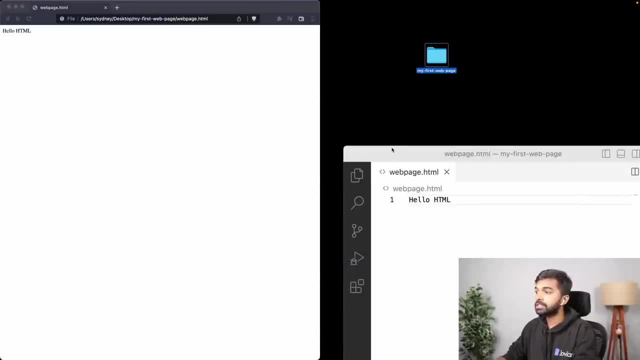 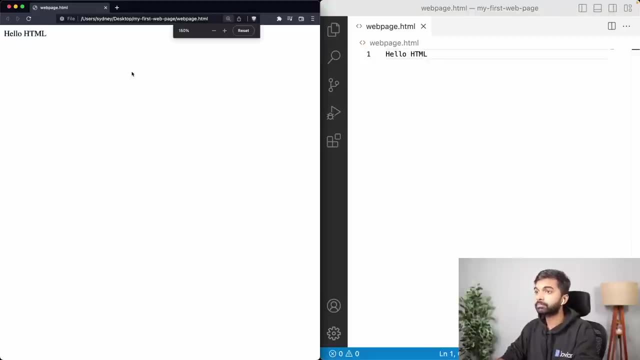 that I'm using And you can see, as soon as I opened it, the same text that I entered into the web page or HTML file, the exact same text, showed up here. You can see. I'm just zooming into about 200% so that you can see it more clearly. 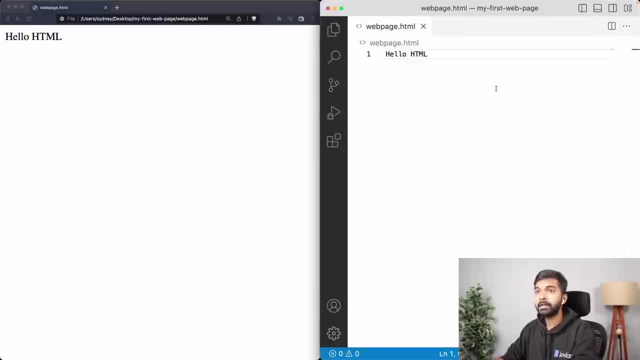 Okay, Let's keep it at 200.. All right, So Hello HTML is what I typed here And Hello HTML is what showed up when I opened. when I opened web page, or HTML in the web browser. So that's it. That's how you create a web page. you just create a text file. call it something. 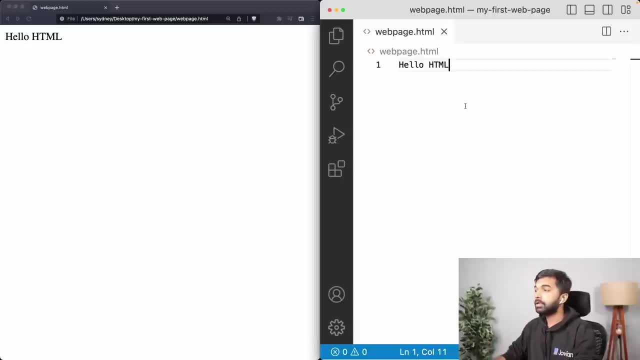 or HTML, and then open it in a web browser and you have a web page. However, you want to put some kind of a structure into the web page, because we don't just want to write text. we can post a lot of text, but it'll all be in the web page. So that's how you create a web page. So that's how you. 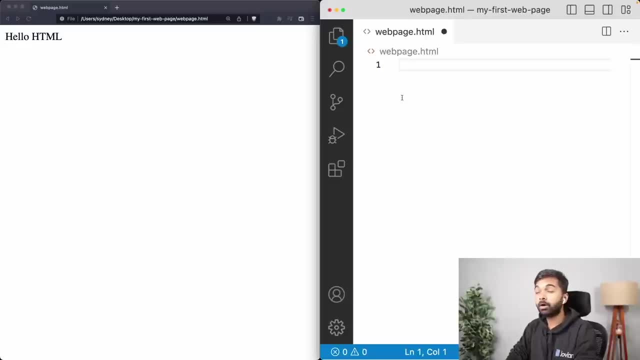 create a web page. I'll just be text on the screen, But that is where you use something called tags. So first let me just put in some code here. So I'm going to create this tag called HTML And you can see that this tag starts with a less than symbol or an arrow bracket, and ends. 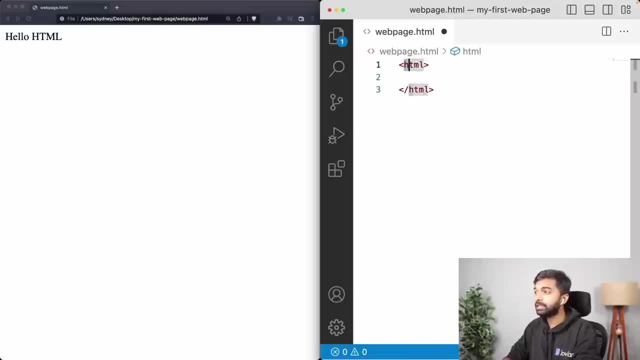 with an arrow bracket And every tag has a tag name. In this case, this tag has the name HTML. let me zoom in further. So it has the name HTML And every tag generally has a closing tag. Okay, So this is the opening HTML tag And HTML is always the outer. 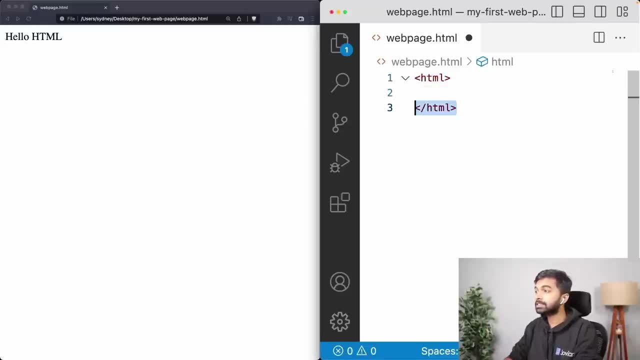 tag in any webpage, And then there is this closing HTML tag, And the difference between the opening and the closing tag is this slash character before the tag name. Okay, So any HTML page or any web page is built up using tags. These tags are used to create structure within the page. Okay Now. 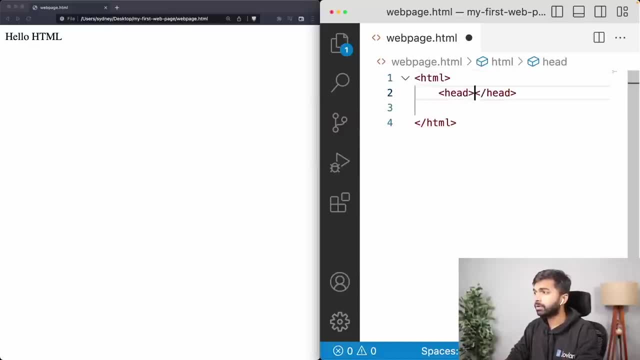 within an HTML tag, I'm going to put in a head tag. Okay, We'll talk about what these tags do in just a second. And again, VS Code does this nice thing that as soon as you create an opening tag, it automatically adds a closing tag for you, And that is why developers use these code editors. 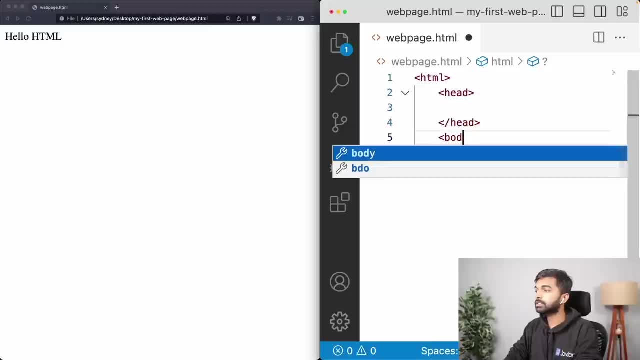 Okay, And then another tag that I'm going to put in here is called the body tag. Okay, So now we have a HTML tag, which is the outermost tag. inside it we have the head tag and the body tag, And let me just save that for a second and reload, And you can see now all the content has. 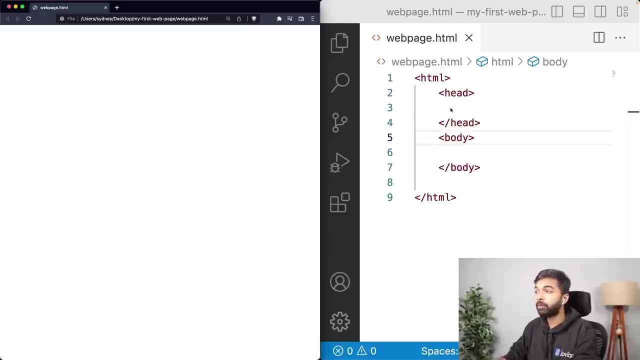 gone away. So now nothing is showing up on the browser because we've not put any content into the page. The first thing I'm going to do is, inside the head tag, I'm going to put in a title tag. Okay, So I've just typed title, I've created an opening tag. 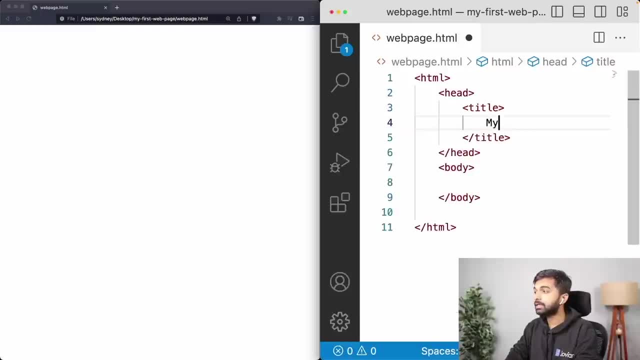 and VS Code added a closing tag for me And let me just say my first web page here inside the title. let me save that. Let me come back here into the browser reload And now you will notice that nothing has happened here on the page. But if you notice carefully the browser tab, 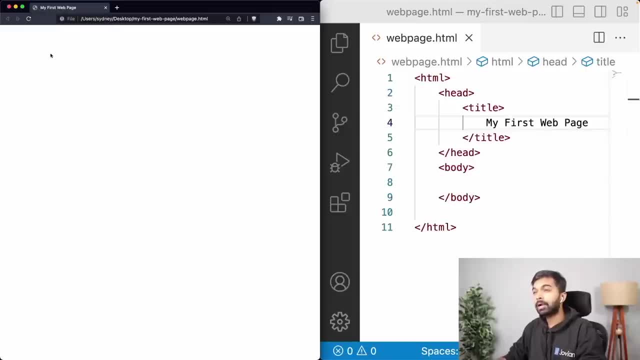 the browser heading, the tab. So the browser tab. here it has the title: my first web page. And now let's come back here to the browser. It says the title hyperlink And I'm going to say that again: title: my first web page. Okay, so it has the title: my first web page and you can zoom in. 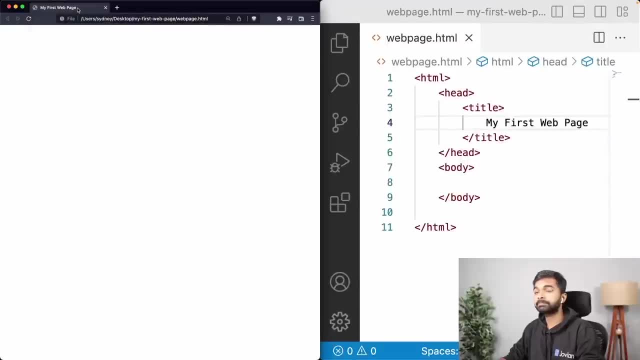 here and I can zoom in here and I can show you that it has. it has a title, my first web page. All right, Now let us add something here in the body. So I'm going to just add something called a div here in the body. So div is again another tag that is used to put. 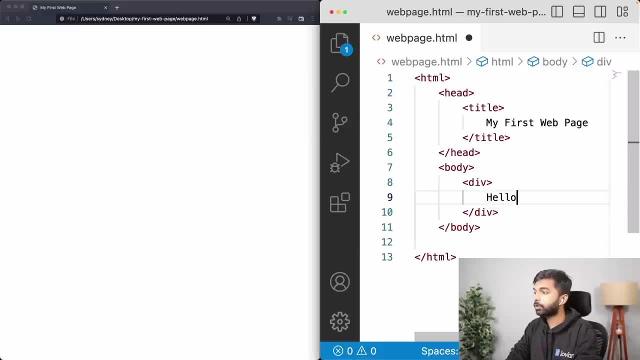 some content into the body And let me just put here: Hello, HTML and CSS. Okay, So this is what a typical web page or a typical HTML document looks like. It contains a bunch of tags, and then it contains tags within tags, and each tag has a specific purpose. Okay, 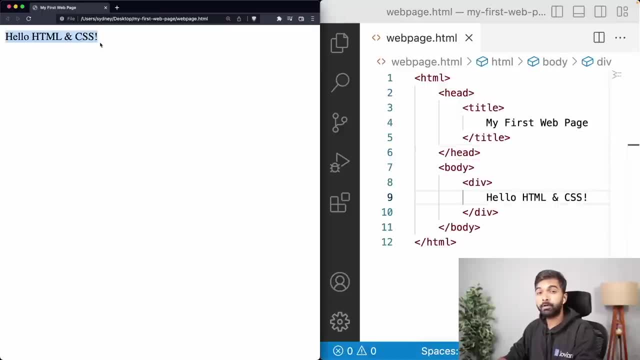 now let me put that in and let me reload. and now you can see that here we have Hello HTML and CSS, And then you can go back and change this. Let's say, let me make it Hello HTML slash CSS and let me reload. 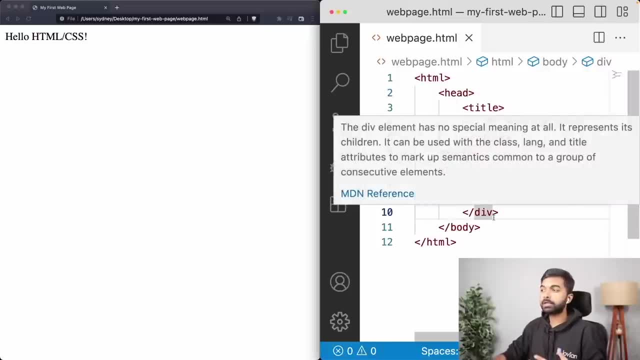 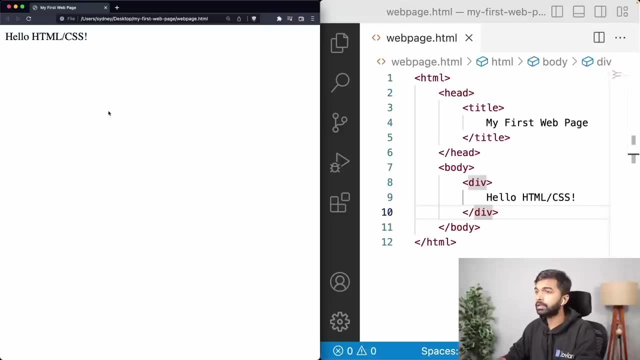 Now it says: Hello, HTML slash CSS. Okay, so this is how you construct a web page. you put in some tags and then you open the web page in a web browser. All right, So that's the basics of how you create an HTML page. you launch VS code. open up the project folder. 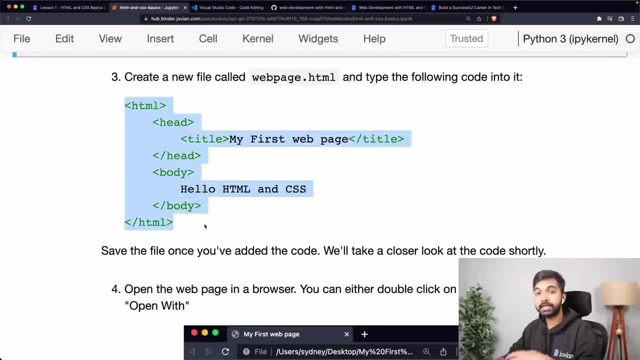 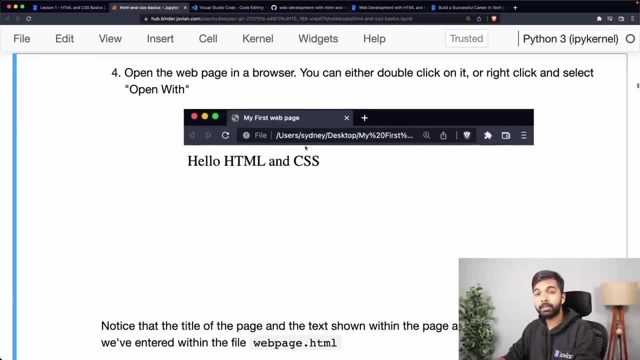 within VS code and then put some code into it. This is HTML code, So we put in an HTML tag head, tag, title and body and then save the file once you've added the code, and then open it with a browser And this is what it looks like. 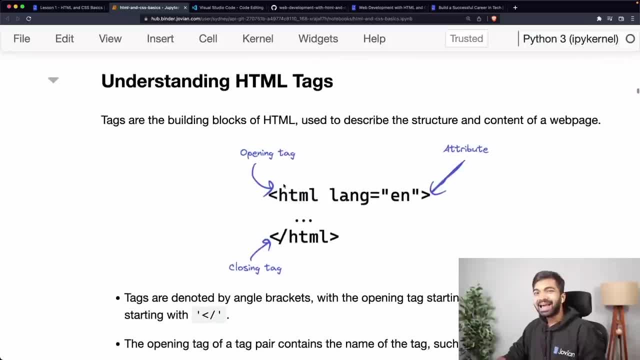 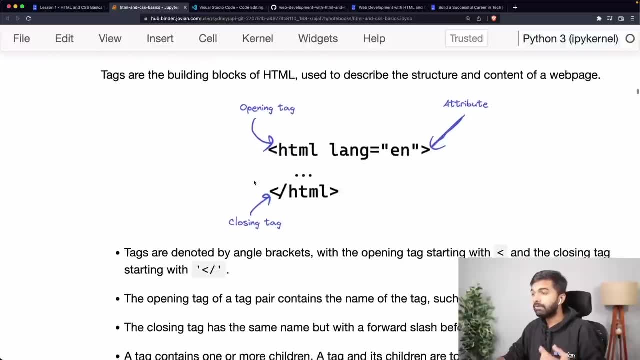 Now let's understand HTML tags a little better. So tags are the building blocks of HTML and they are used to describe the structure and the content of a web page. Now, normally every tag will have an opening tag, like the HTML tag had an opening tag like this over here: 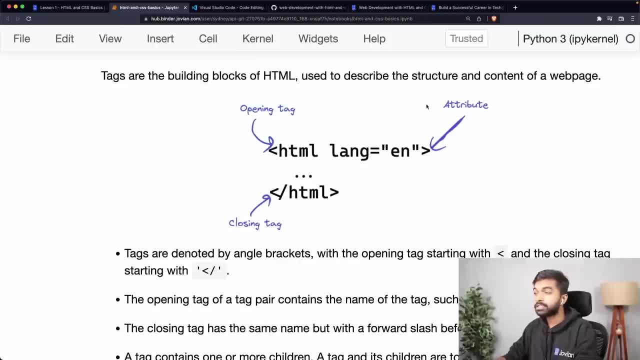 And it will also have a corresponding closing tag. And sometimes tags can have attributes and these attributes are used to provide more information to the browser or modify the behavior of a particular tag. For example, the HTML tags are used to provide more information to the browser or modify. 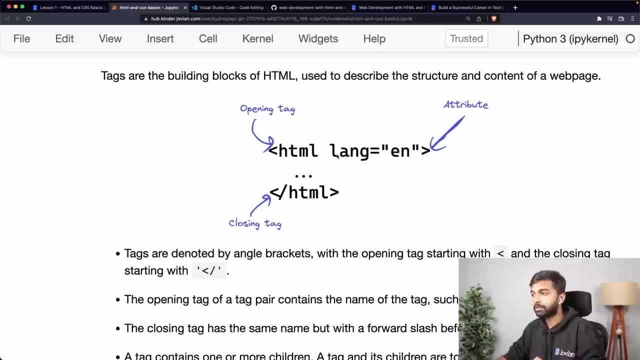 the behavior of a particular tag. For example, the HTML tags are used to provide more information to the browser or modify the behavior of a particular tag. So the tag has this attribute called Lang, which is simply written in within the opening tag itself, And then the attribute Lang is given a value en, which means English. So here: 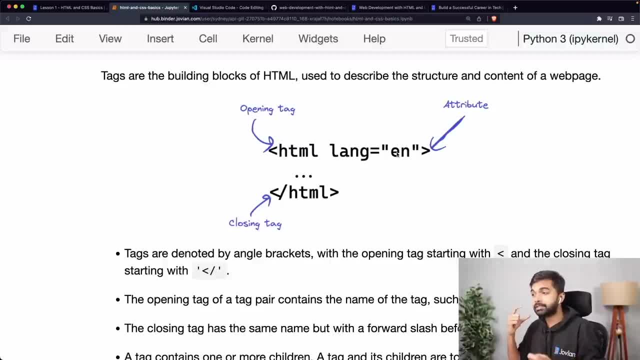 what we're doing is we're indicating to the browser that this particular HTML page is written in the English language, So now that browser can use it for, let's say, setting up a translation, automatic translation tool or something like that. right, So an attribute. 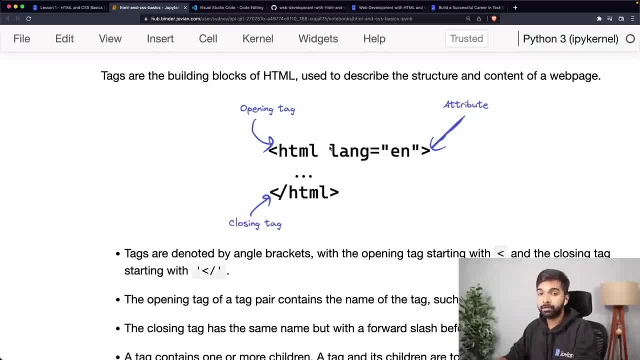 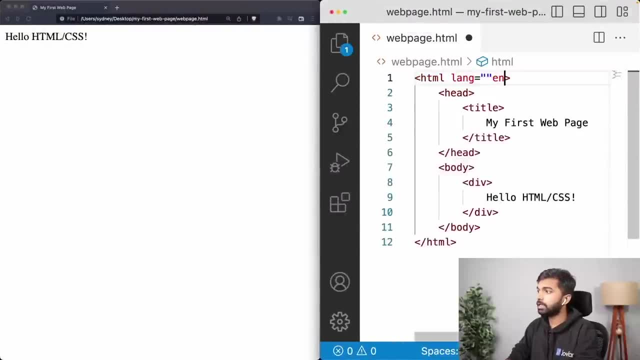 is used to provide some additional information about that tag or modify the behavior of that tag. So then we look at a lot of attributes with time. So I can say here, for example, HTML Lang equal to en And that doesn't do anything visible, But that does inform the. 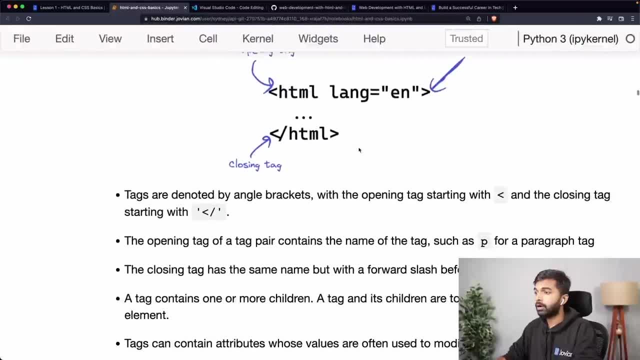 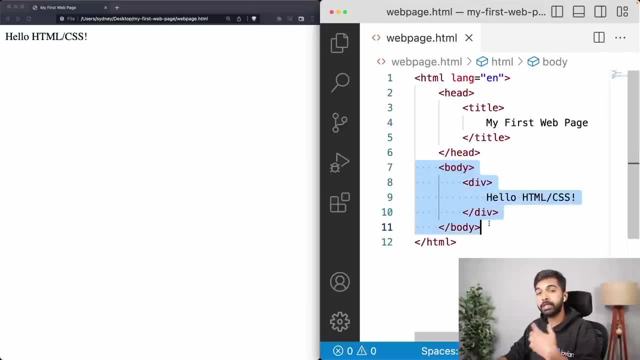 browser that this is an English web page. All right Now. so that's about tags, and a tag can contain one or more children, So like the head and the body are called the children of the HTML tag, And a tag along with its children together is called an element. 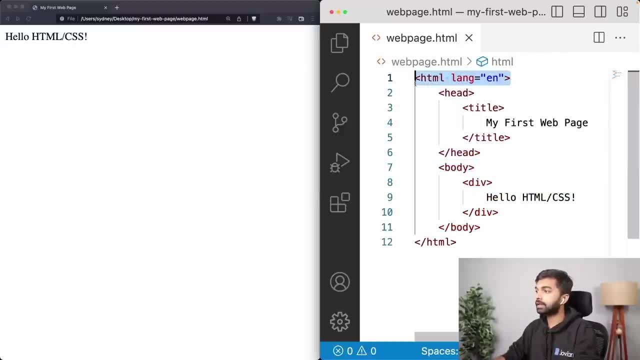 Okay, so the tag is simply this piece. This is the opening tag and this is the closing tag. Everything inside a tag is called its children, which is again other tags, And then a tag together with its children is called an element. So this whole thing is an element And then this is an element. 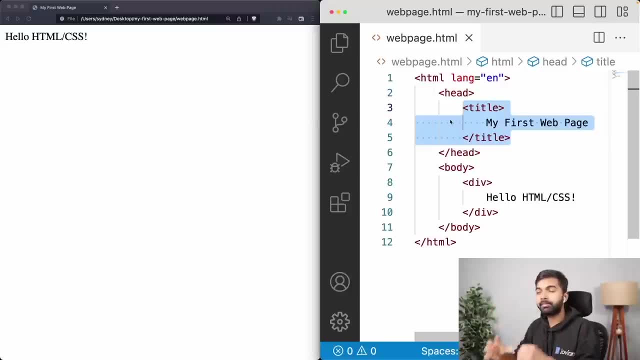 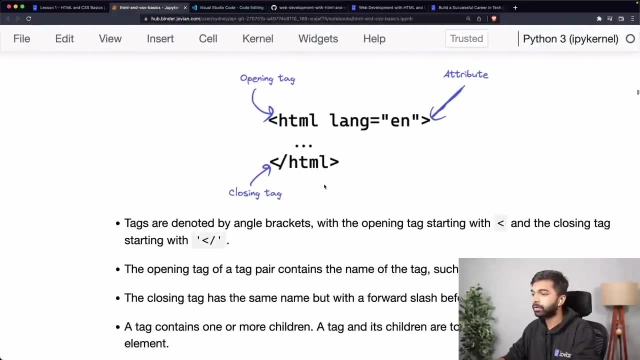 And then this is an element. So every tag, along with its children, is an element. And then what's a? whatever the inside, a tag is called children. okay, these are just some terminology that you will see when you're reading about HTML and CSS. All right Now. 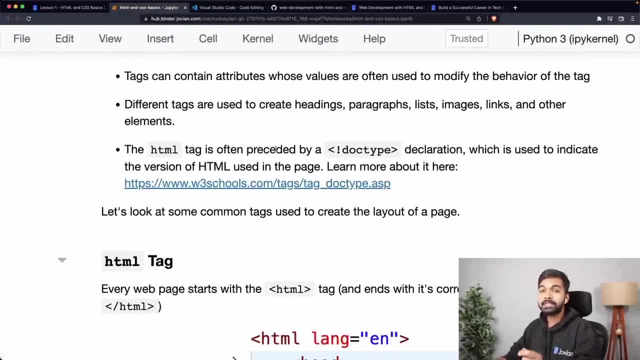 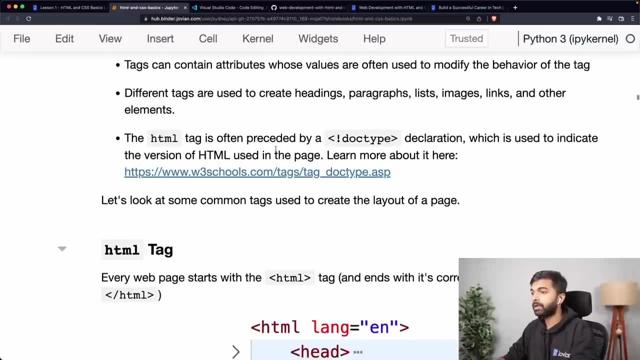 tags contain attributes. we talked about that, that- and there are various tags, So let's look at that. And there are various different tags to create headings, paragraphs, lists, images, etc. And we look at those in just a bit. Now, one thing I want to mention is: 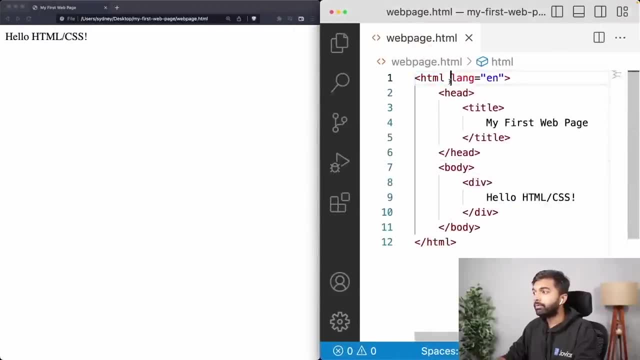 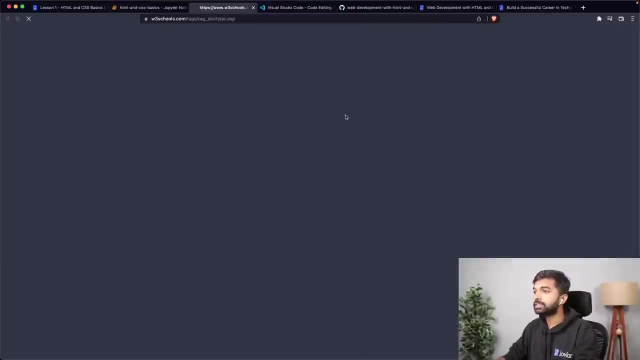 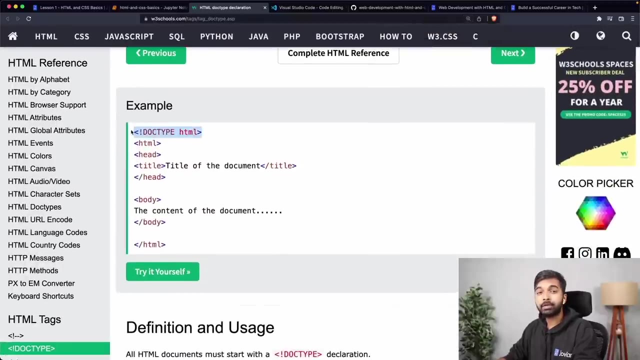 that HTML is the outermost tag. However, in many web pages you will find a doctype declaration just above the HTML tag, So you will find something like this: you will find a doctype. let me zoom in here, So you will find doctype HTML at the top of most web pages And you. 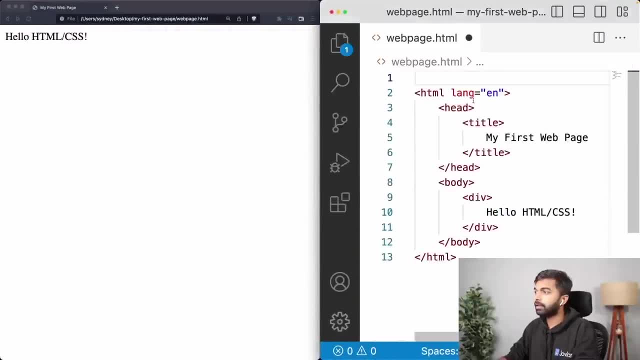 can just copy this and put it at the top of each HTML page And that is just a good convention that is followed, that at the top of every HTML web page it's a good idea to just put this doctype HTML, okay, And this: this is just something that you copy paste at the 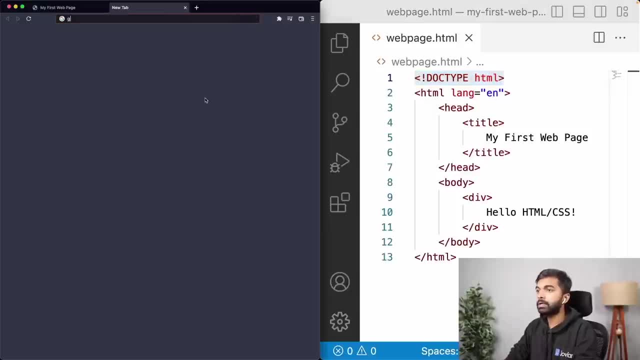 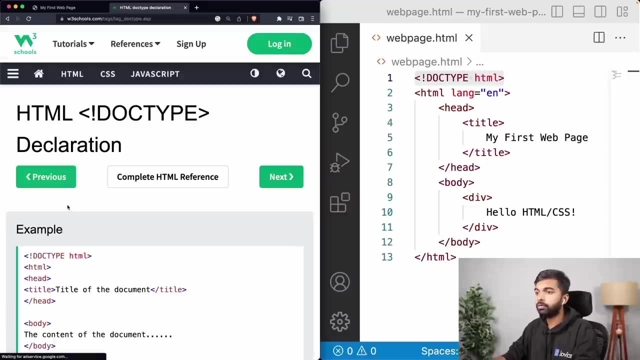 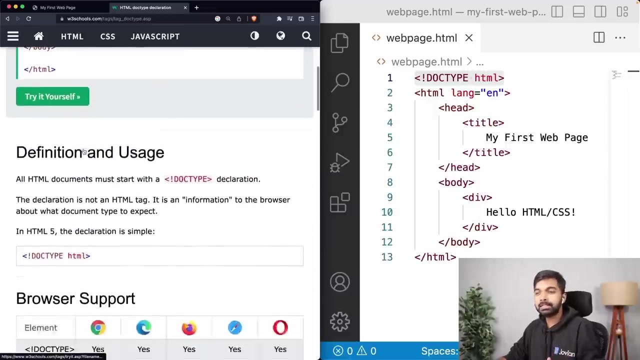 top of every HTML web page And you can literally just go on Google and search doctype declaration. Okay, And you can find this link- HTML doctype declaration- and you can just copy this and put it at the top of each HTML page And if you want to understand what this does, you. 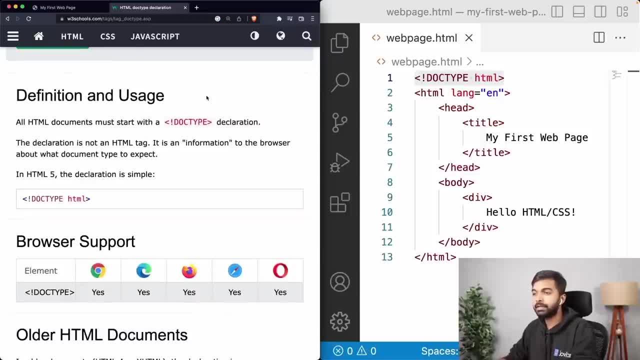 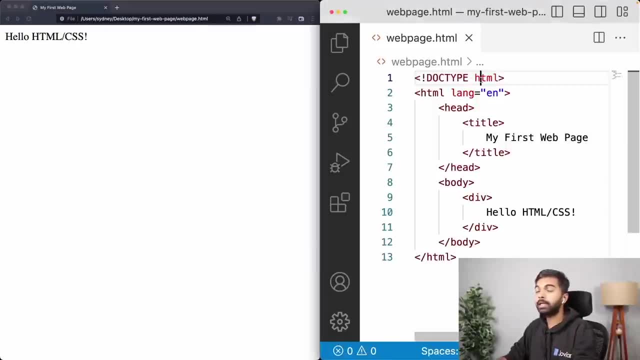 can I encourage you to go through this h w three schools link. It's not important, It's just a convention that you want to put in because there have been multiple versions of HTML And this is a way for you to indicate that you want to use the latest version of. 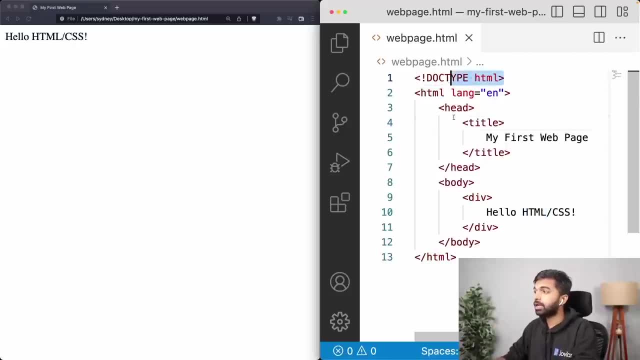 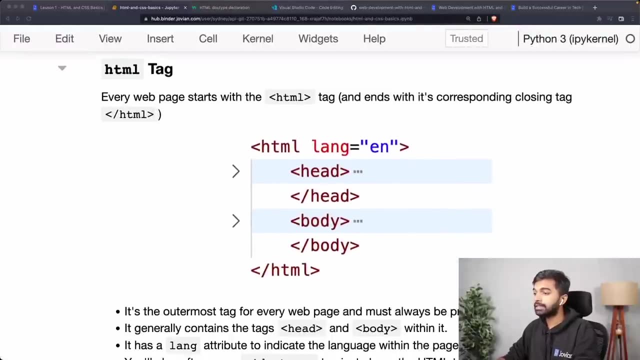 HTML to the browser. Okay, now we have the doctype, then we have a bunch of these tags. The HTML tag is the outermost tag- we already talked about that- And the HTML tag is typically only contains two other tags- the head tag and the body tag- And it has a lang attribute. 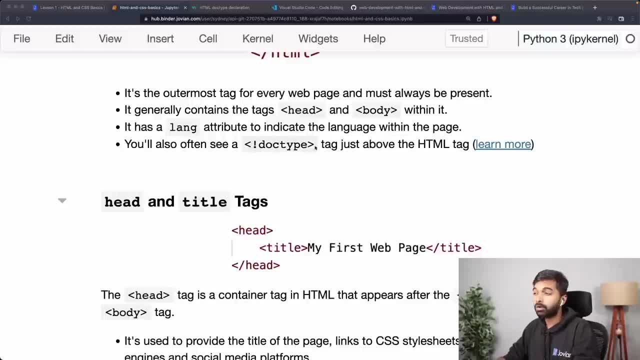 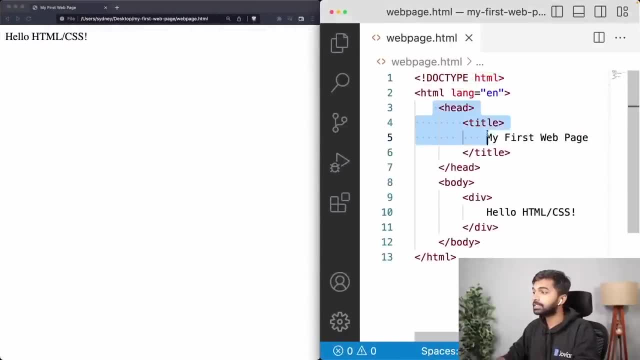 and it has some other attributes also that can be set And you will see a doctype declaration just above HTML. So that's the HTML tag. Okay, then we have the head and title tags, which are the tags that we are seeing here. So the head tag is a container tag in HTML that often 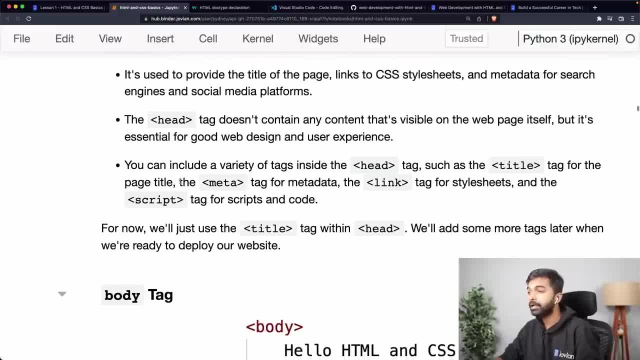 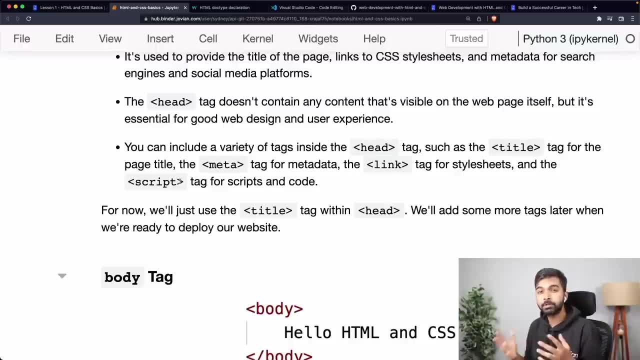 doesn't contain any content that is going to be visible on the page exactly, But it generally contains some information that is passed on to the browser And that is useful for the browser, And that is also useful when you're sharing this link with somebody else. 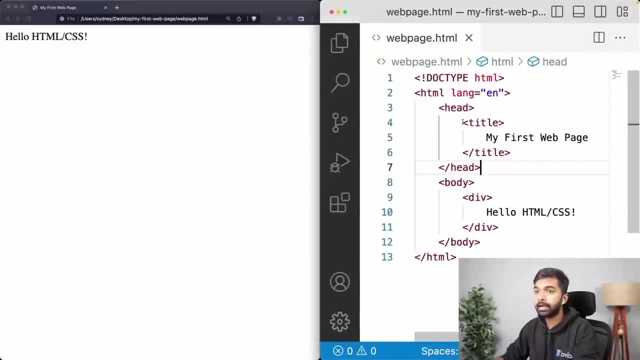 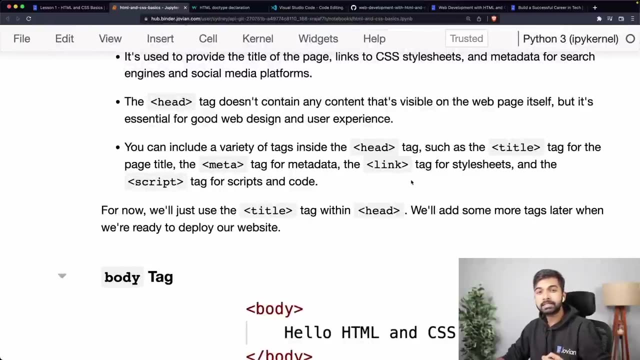 So, for example, it contains the title tag. we put in the title tag over here in the head, And the title tag is used to set the title of the browser tab. Similarly, there are some meta tags, so, and then some meta image tags, etc. And these are used to set the preview. 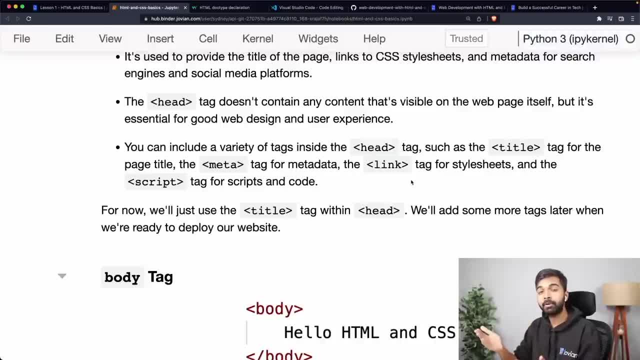 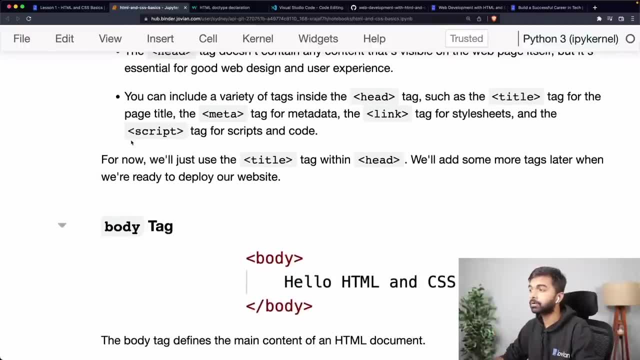 image and the description that shows up when you share this link on a social platform or when this is seen by a search engine or something like that. Okay, so the head tag is very useful. It is also used to sometimes include maybe style sheets, CSS files, and sometimes used. 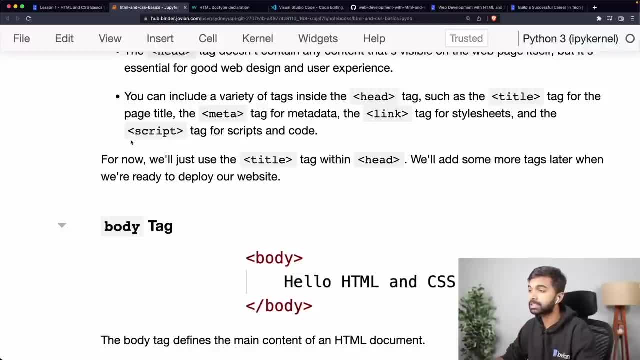 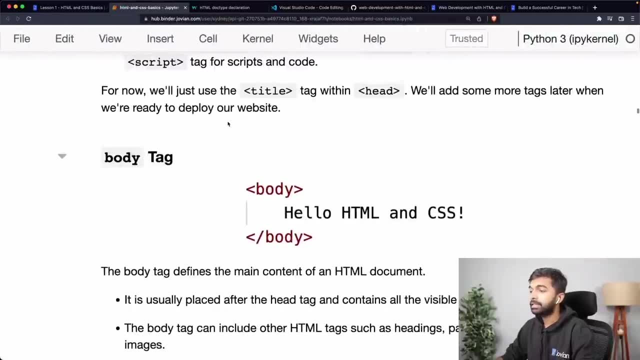 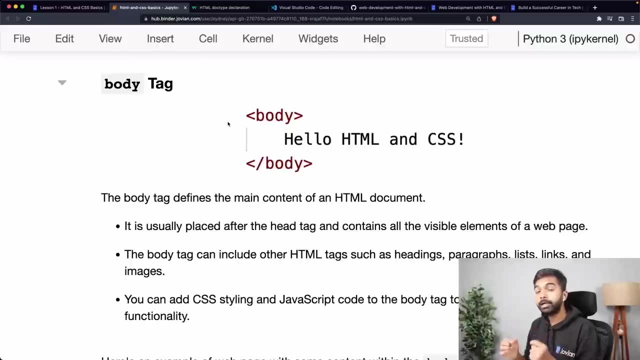 include scripts. we'll cover all of these. don't worry if these terms don't make sense just yet. for now we're just using the title tag within head. so within head we just have the title tag and then we have the body tag. now, within any html page, you have a body tag and the body tag defines: 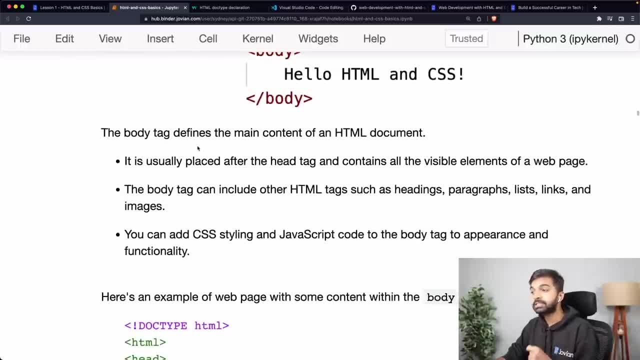 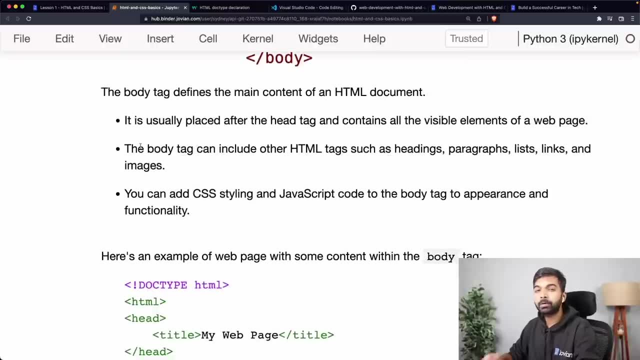 the main content of the html document. it is usually placed after the head tag and it contains all the visible elements of a web page. okay, and the body tag can also include other html tags like headings, paragraphs, links, etc. and here is the key thing, here is the key difference between just 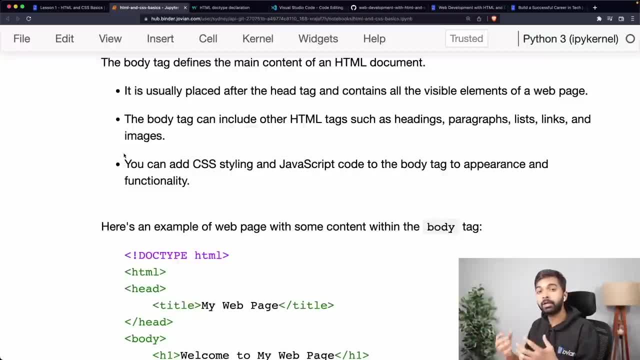 putting some text into a file versus putting it in the body tag and putting it in in html tags. you can add styling, you can add colors, fonts, you can change the layout and you can even add interactivity using javascript and css. right, so all of these things are applied within the elements. 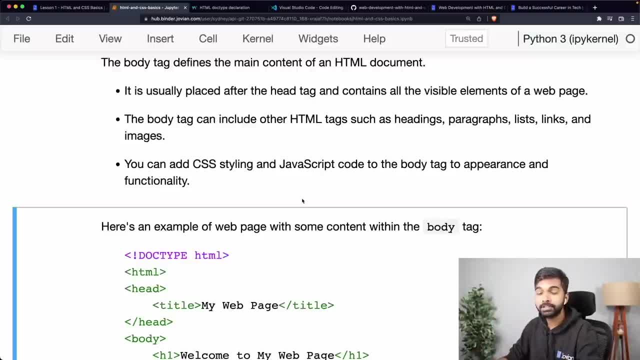 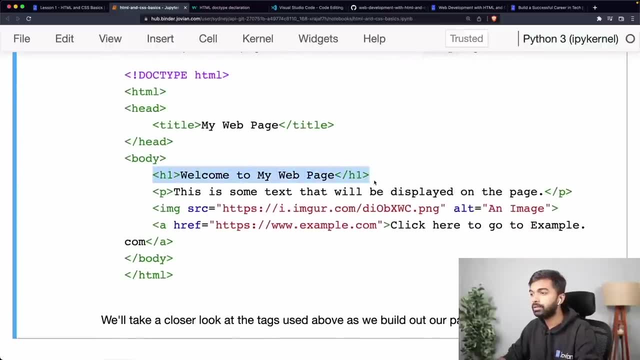 in the body tag to change the appearance and functionality of the web page. so here is an example of a web page with some content within the body tag. so here there is an h1, which is a heading tag- we'll talk about it. there is a paragraph tag. there is an image tag. 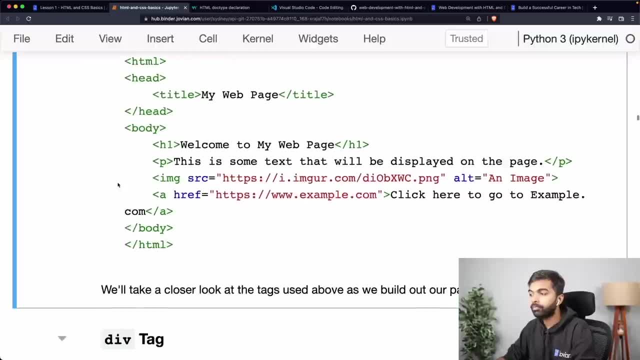 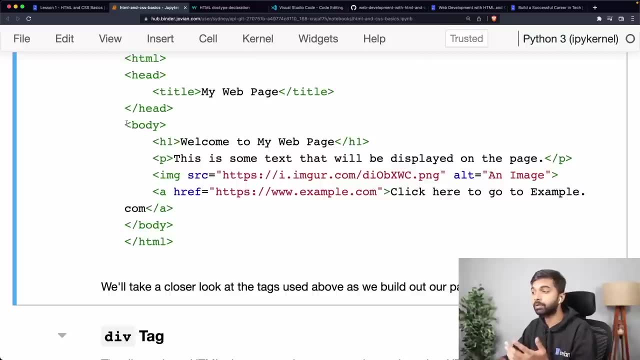 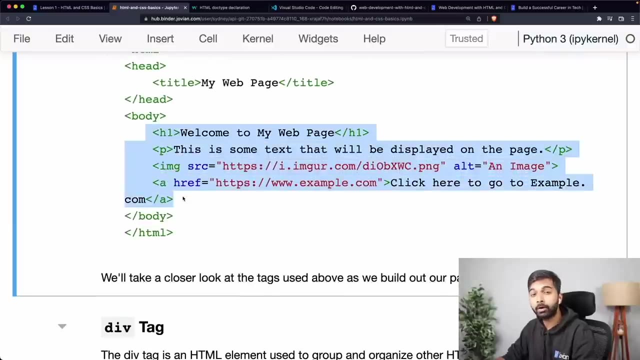 and there is a a tag, so i will not paste these right now, but i'll actually leave these as an exercise. so maybe just try and paste this into an html page, open it in the web browser and see what you can come up with. okay, so that is the body tag. it is what contains all the content of the. 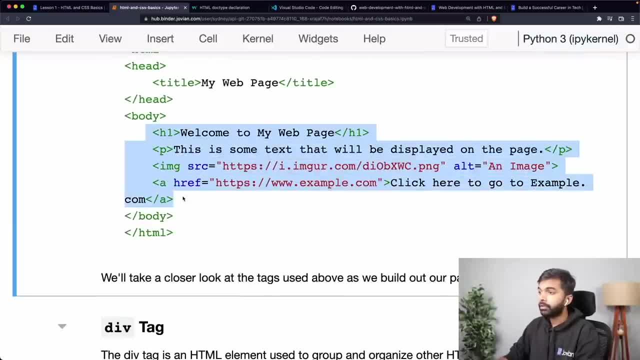 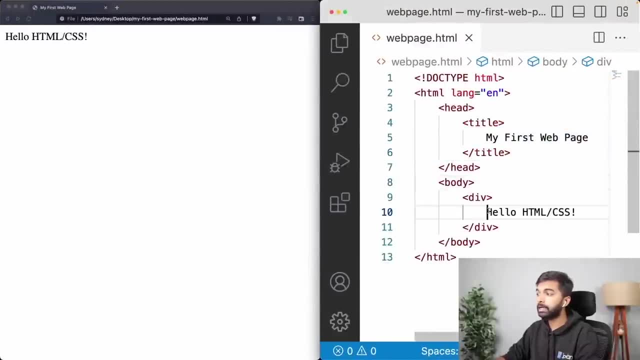 web page that we are going to be building today. then we have the div tag. okay, now you notice that inside the body i did not directly put in hello html css. i created a div so i didn't have to do this. i could have just put it into the body itself, but the div tag is typically an html element that. 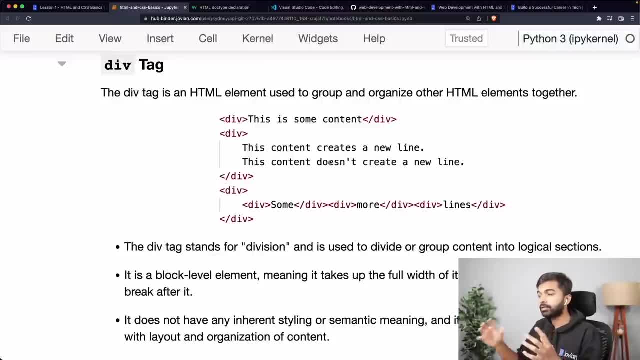 is used to group and organize other html elements together. for example, you can create one one piece div, div. this is some content, and then you can have a second piece of content under in the second div, and then you can have maybe a third piece of content which is itself divided into multiple. 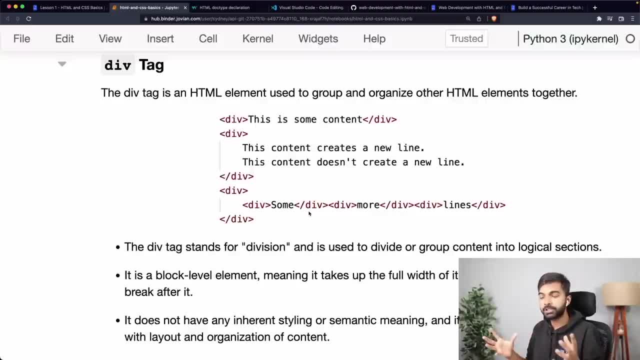 pieces of content in this third div. okay, so div stands for division and it literally creates a division on the page vertically speaking. it kind of divides the page vertically, essentially, you can think about it, and it is used to divide or group content into logical sections and it is a 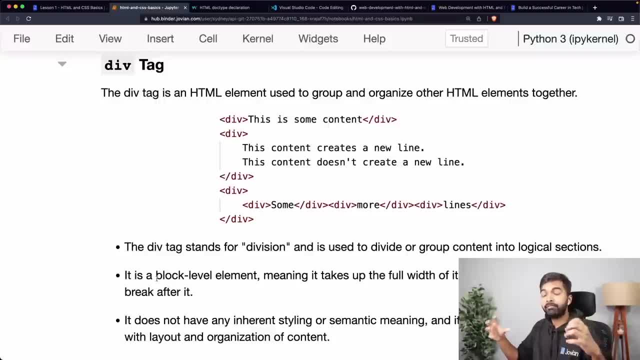 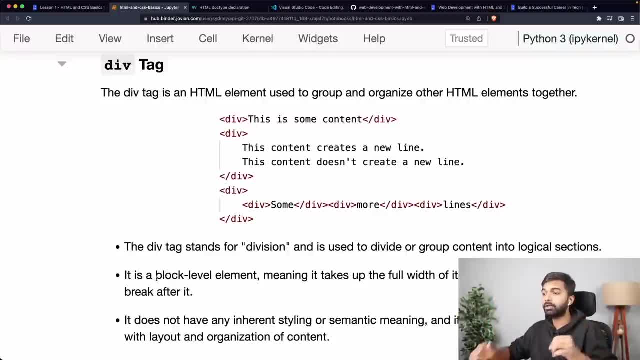 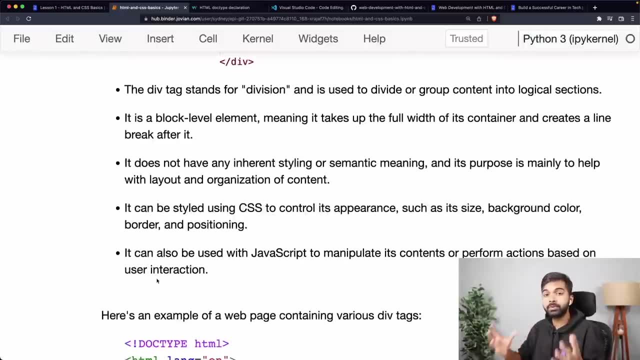 full width, and then the next div tag takes up the full width, and then the next div tag takes up the full width. next div tag is going to appear below it, and the next div tag is going to appear below it, and so on, and it does not have any its own style or semantic meaning or anything, but it is used with css for. 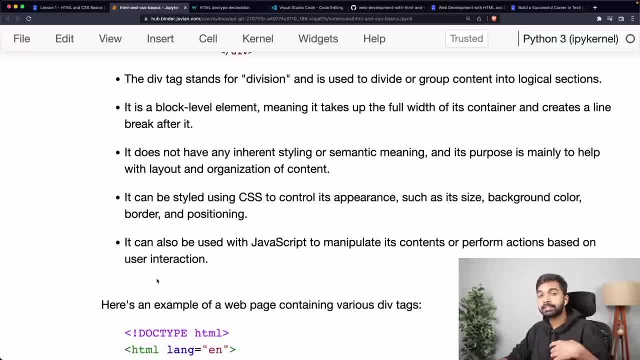 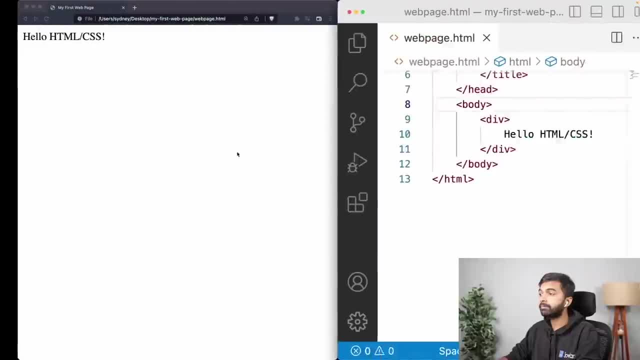 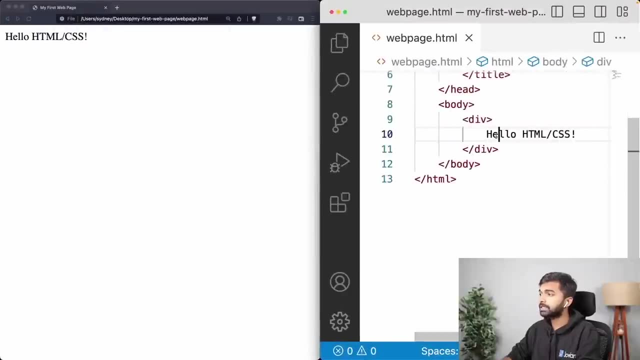 styling. okay, so the div tag is something that we will attach a lot of css properties into to style the web page. so let us create a. let us look at an example of a web page containing some div tags. okay, so here is the content that we're going to put in, or type in one by one. so first let us create a div. 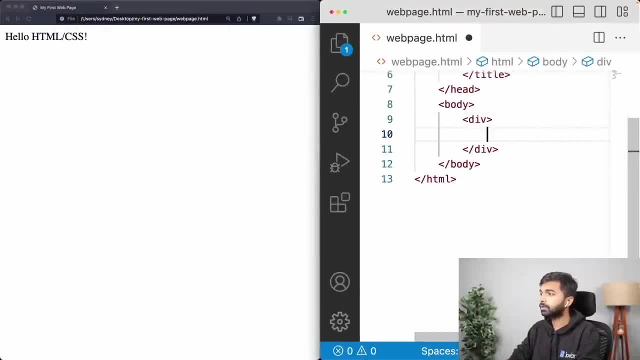 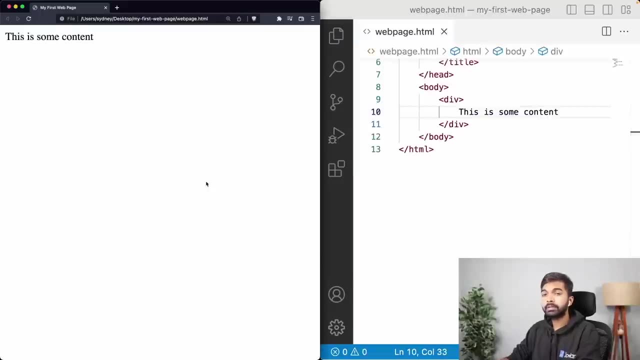 tag and let us say: this is some content. okay, so now we have put in some content div tag and it says: this is some content, as we might expect. then let me create another div tag and let me say: this is a second line of content. okay, now, if i reload the page, you will notice that this content showed up below this content. 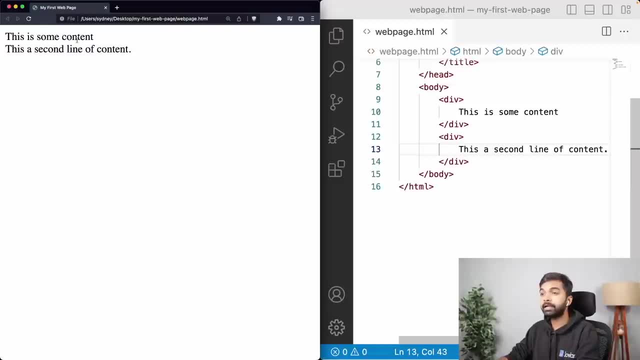 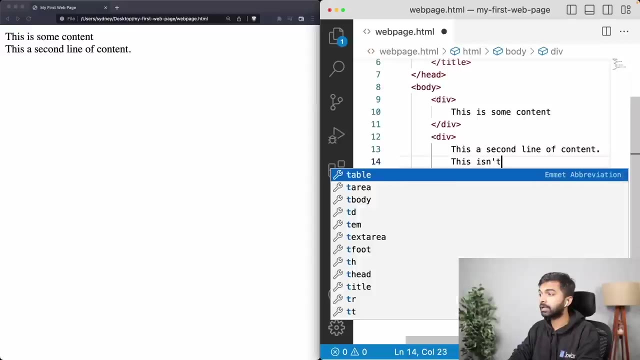 So that is what the div tag is creating. it is basically creating a division within the page, So this content is shows up in this area and then this content shows up below it in this area. Now notice that I can go into the next line I can type. this is isn't a third line. 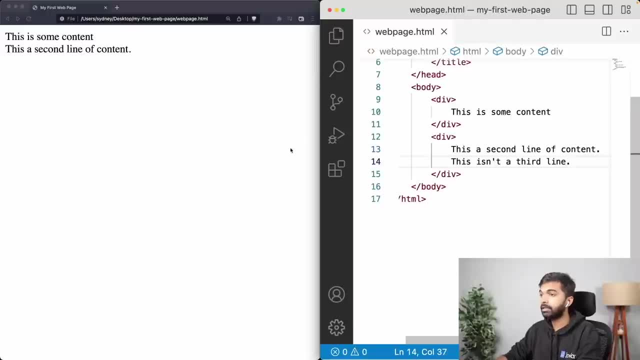 Now, I'm not creating a new div tag. I'm still using the second div tag, But this time you can see that even though I've typed this content on a new line, it is still showing up on the same line as the second line. Okay, so here is the important. 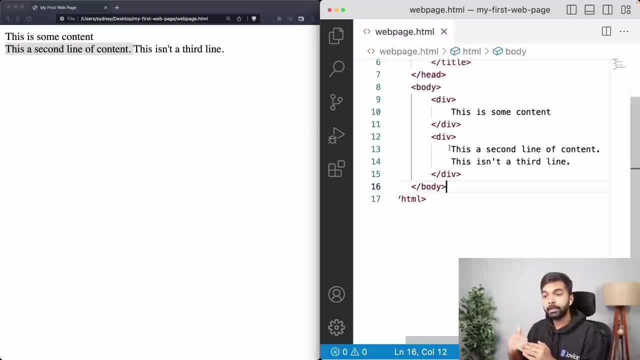 importance of div. If you want to split content vertically on a on a web page, then you want to create divs and each div is going to create a new vertical section or new vertical division within the web page. Okay, And if you simply create multiple lines of content like this, all of that? 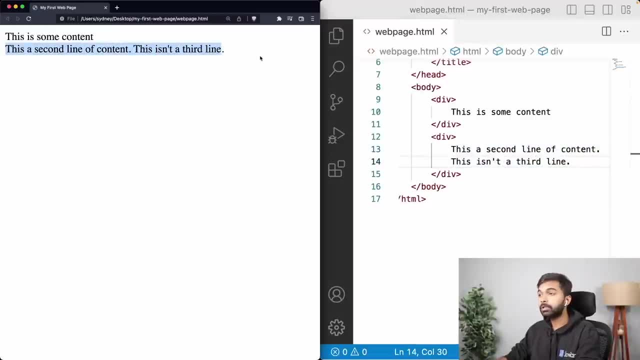 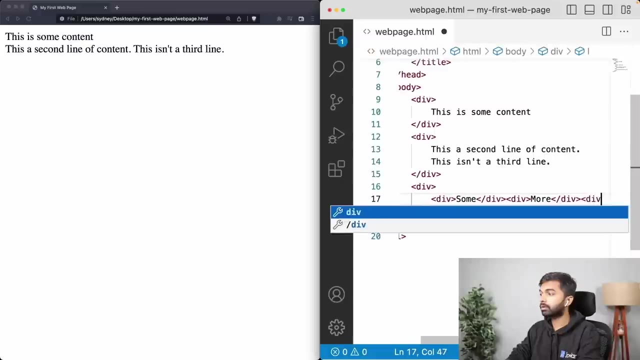 is going to show up in a straight line. that is not necessarily going to show up one below the other. Now here is another example. Now this time I have a diff div tag, but inside the div I'm then creating more divs. So some more lines, Okay. 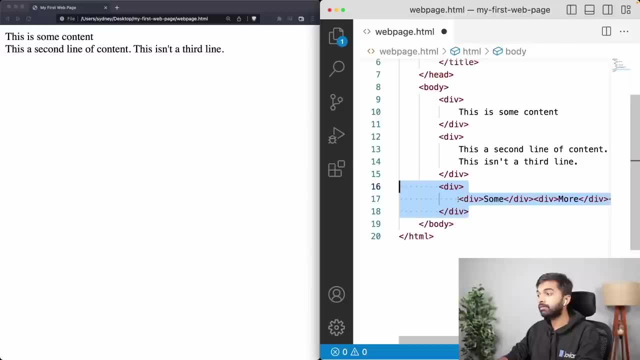 so now I have this third div tag, And now, in this third div tag, I have again another div tag, three more div tags, one around each word. But now, even though all these three div tags are on the same line, within the HTML source code, you can see that each div, each inner div tag, 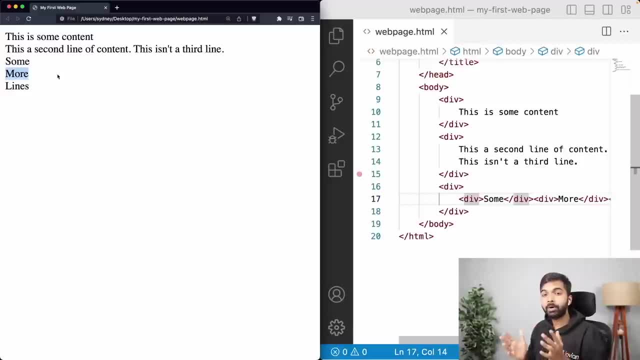 up its own vertical space. Okay, So that's what I want to convey here: that as you want to keep building, as you want to keep adding content below the existing content on a webpage, you should be creating new div tags. So that is the div tag. 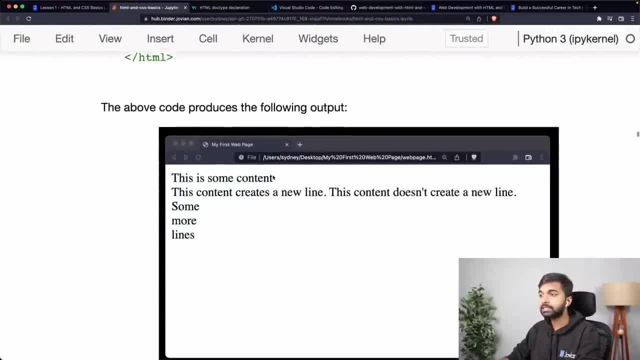 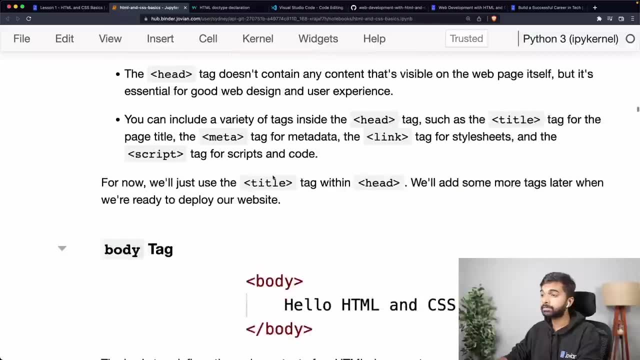 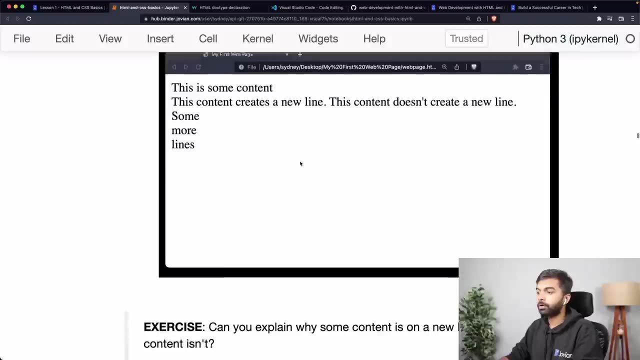 And those are the most basic HTML tags. Now, we've just looked at what the head, the HTML tag. we've looked at the head and title tags. we've looked at the body tag, we have looked at the div tag and I'll encourage you to experiment with this, what we really want to do. 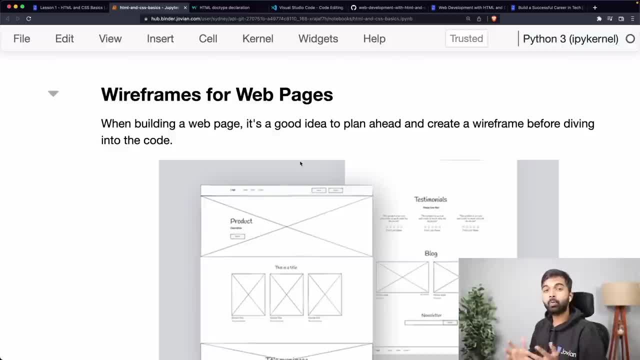 though, is maybe first figure out what our web, what we want our webpage to look like. Okay, So when, when you're building a webpage, it's a good idea to first plan ahead and create what is called a wireframe, And this is what a wireframe for a webpage look like. 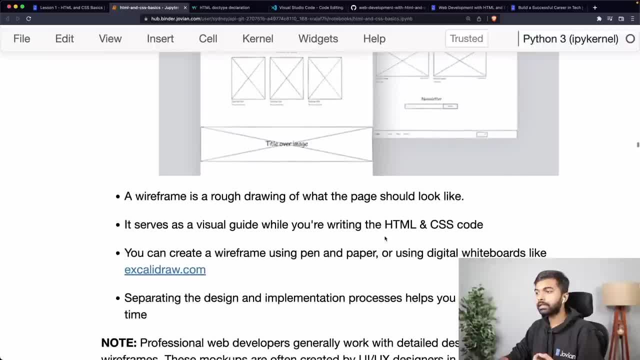 It just. it is just a rough drawing of what the webpage should look like. Okay, That's what we typically call a wireframe. Like You don't put in colors, You don't put in exact fonts and sizes of fonts, et cetera. 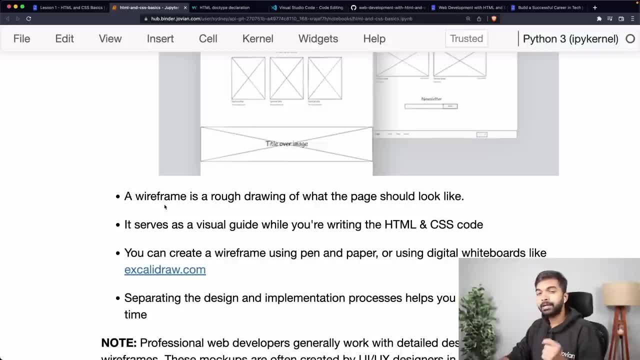 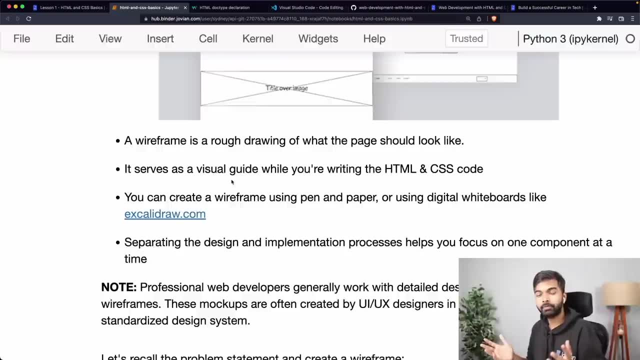 You just put a rough diagram of the structure of the page and you can use that as a visual guide while you're writing the HTML and CSS. Okay Now, if you don't already have a design to work with, then sometimes it can be. 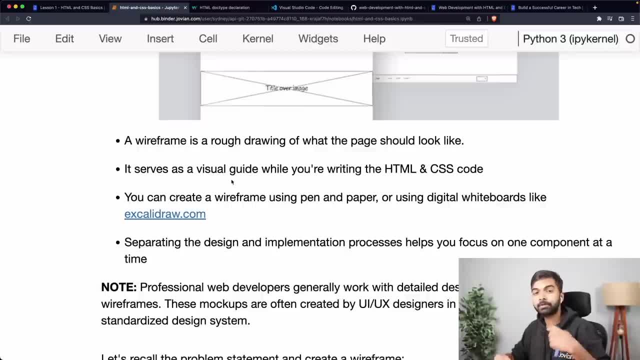 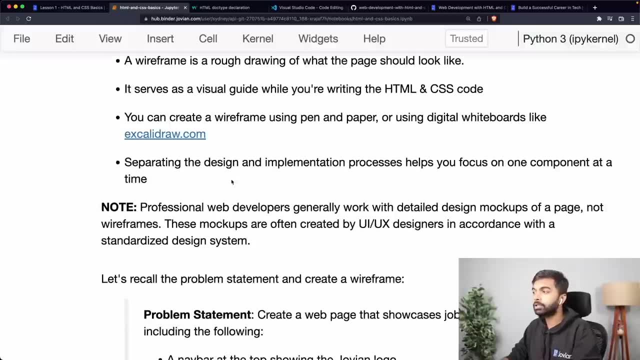 confusing if you're trying to design your webpage as you're trying to code it. So the having a wireframe is going to help a lot And you can use. you can create a wireframe using pen and paper or you can use digital whiteboards like. 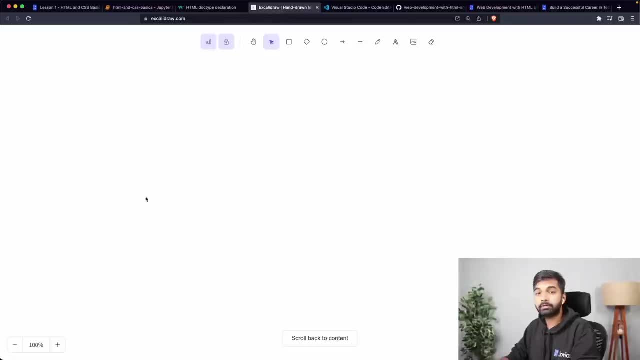 Excaliburcom. So Excaliburcom is a digital whiteboard, So this is what it looks like And here on this digital whiteboard, you can create boxes, You can create circles, You can create lines, You can add text and you can do a bunch of things to create your wireframe. 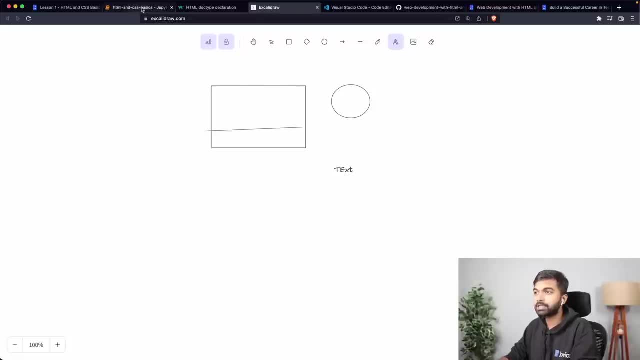 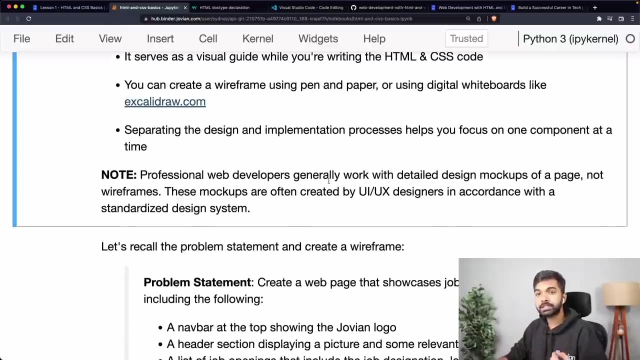 Okay, So you can use a digital whiteboard any- any one of your choice, but I like using Excaliburcom. Um, and the idea here is to separate the design and the implementation process To help you focus on one aspect of the development at a time. 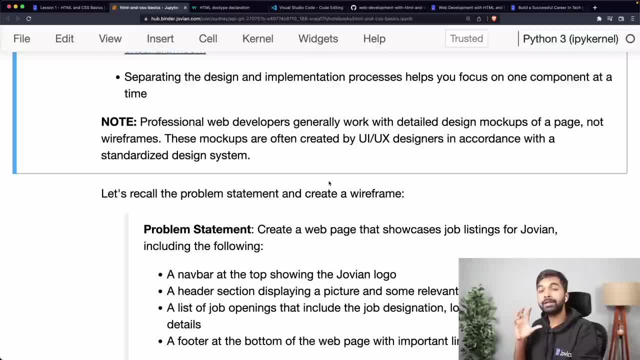 Now. I will note, however, that professional web developers work with a detailed design mock-up of the page and not generally wireframes, because these design mock-ups or these design specifications are often created by UI UX designers with a standardized design system. So normally at a company you will receive a full flesh design and the 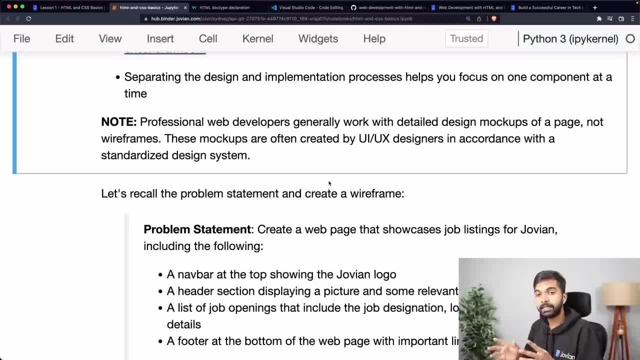 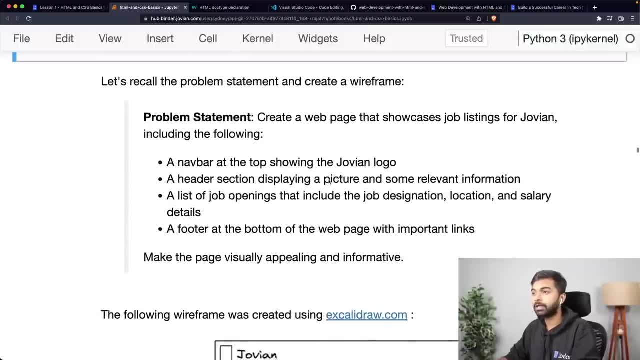 design will have all the colors, all the fonts and everything specified there And you will be working from. But for your own personal project it's okay to maybe just do a quick wireframe and then figure out the design over time, Okay. 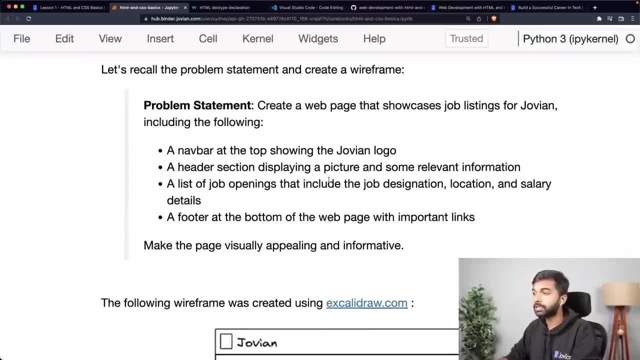 So let's recall the problem statement and then create a wireframe for the problem. We want to create a webpage that showcases job listings for Jovian and it includes a nav bar at the top of the page showing the Jovian logo. it includes a header. 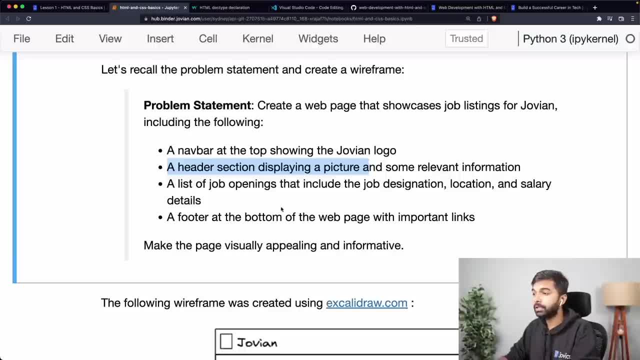 section displaying a picture and some relevant information. then it includes a list of job openings that includes the job designation location, and then it includes A footer at the bottom of the webpage with some important links. Okay, So, keeping these requirements in mind, let us try to first design very broad. 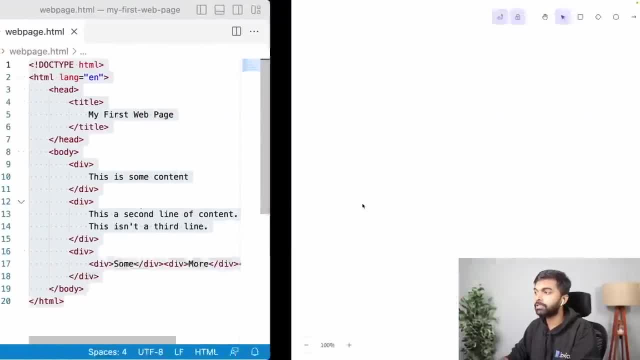 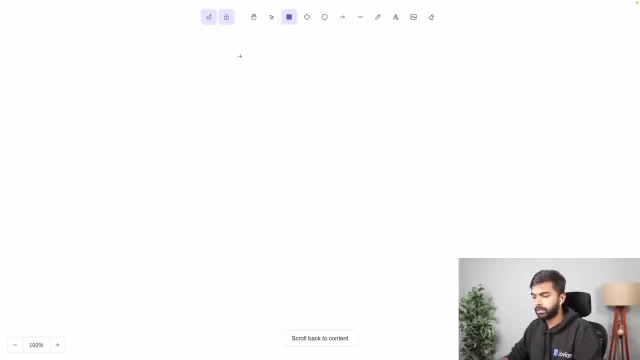 very rough. in a very rough fashion. Let's try to design what this webpage should look like. Okay, So I'm just going to zoom to an area of Excalibur where I can actually design. Now you might see a bunch of these controls here. 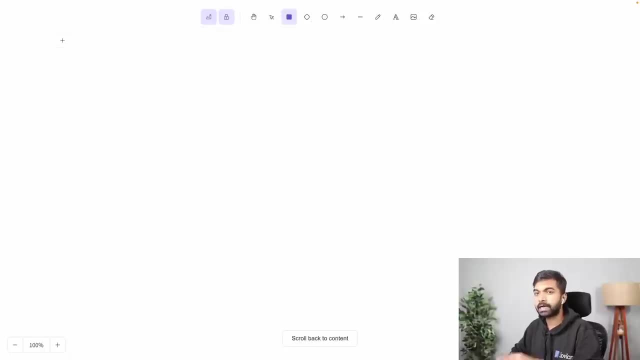 So when you're actually drawing, you might have these controls and you can always hide them. So there's an option called Zen mode here. Uh, but yeah, let's say This is what our webpage is going to look like. Okay, 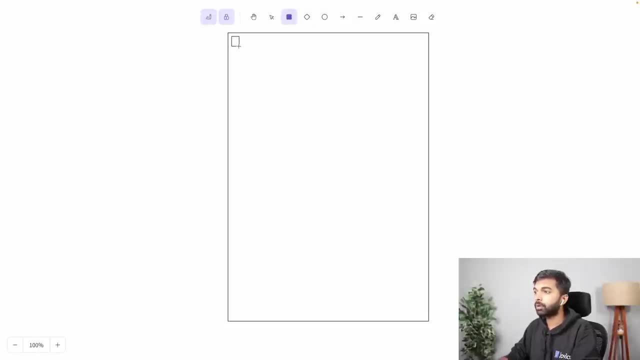 Now at the top of this webpage, we want a Jovian logo, So I'm just going to put a box here indicating the Jovian logo and I'm just going to put the word Jovian here. All right, And so now that's the Jovian logo that is going to show up at the top of the page. 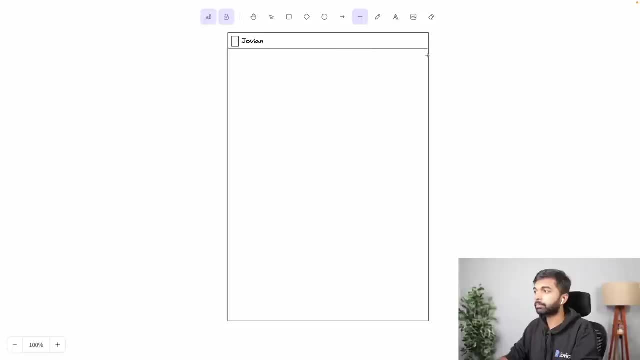 And this is going to be the navigation bar, So maybe let me just put a Separator between this and the rest of the page. then let us- uh, we want maybe a banner image, a header Section with a banner image and some information about Jovian. 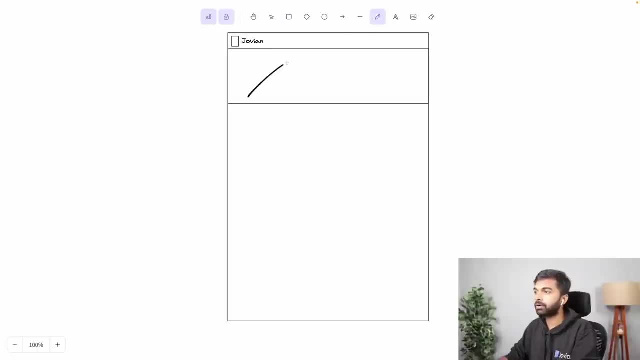 So let's say, this is going to be an image, So I'm just going to draw maybe like some Hills here. Uh, we'll figure out something better than a Hills and a sun, but here we're going to put, here we're going to put an image and then below the image maybe we could have a section called about Jovian, because when somebody visits our job, they job page. we also want to tell them a little bit about Jovian. 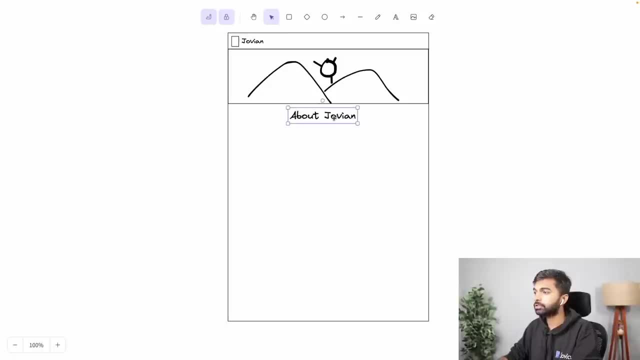 So let me come in here and let me just put in about Jovian And then, uh, maybe on the left here we want a picture of the team. So here we're going to have a team picture- maybe a bunch of people here. 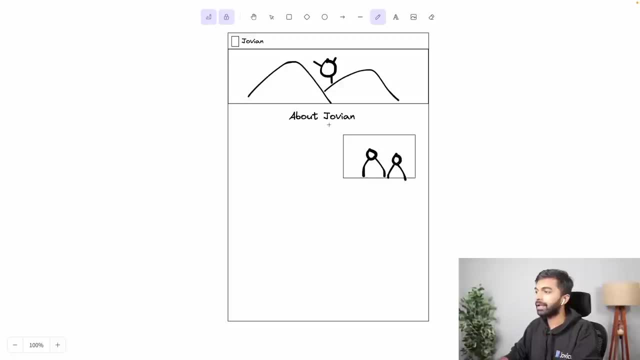 All right, Very, very rough drawing, and here on, on the right, here and on the left, maybe we have some information about Jovian. Okay, So some info about Jovian. Now I'll show you a quick trick. Sometimes you need to generate a, or you need to get a bunch of texts to fill the page. 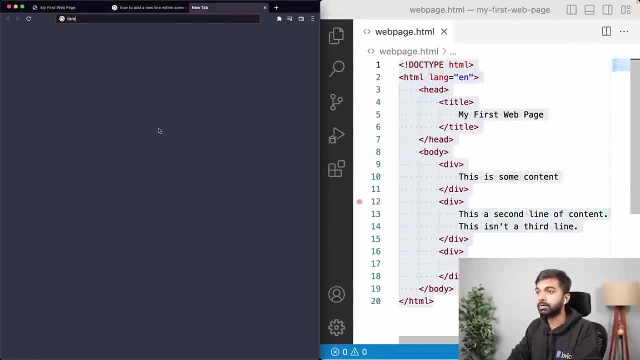 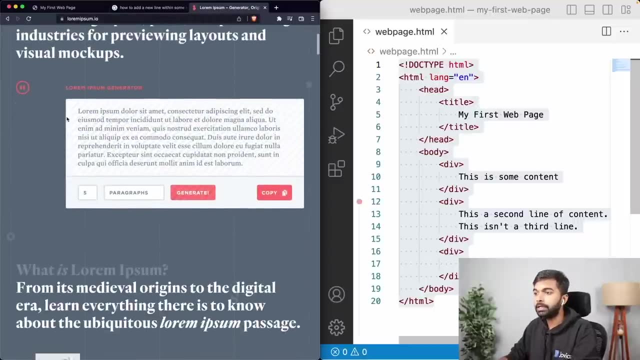 Now that you can do using this tool called lorem ipsum. So lorem ipsumio- Okay, Lorem ipsumio, And the link is in the notebook- is a quick tool to generate as much text as you need, as many paragraphs of text as you need. 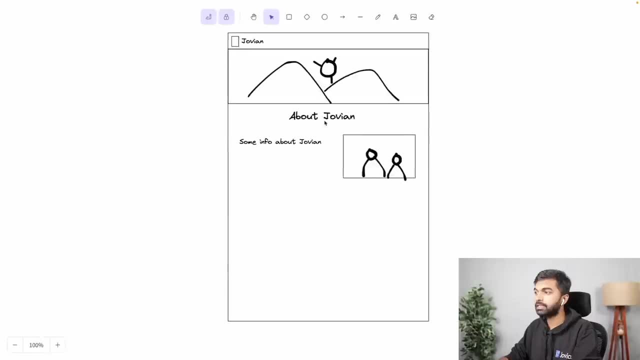 So I'm just going to copy a bunch of this random text. This doesn't mean anything. I'm just going to put that in here and let me just split it into multiple lines. Okay, so yeah, just about that, and maybe also let me just reduce its size a little bit. 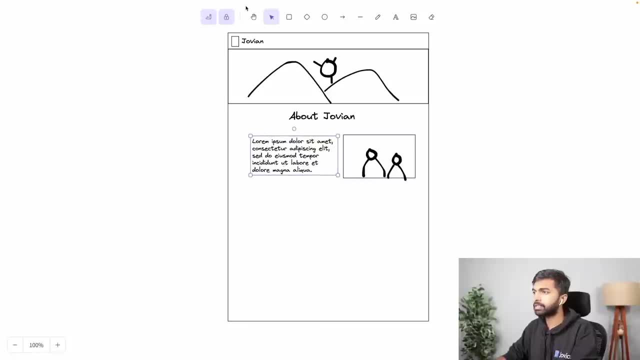 So now we have this, let me change its color. Yeah, Now we have this about Jovian section, this nice about Jovian section over here, and let's move all this here as well. So one nice thing about digital whiteboards is you can move some of this stuff around, and then let us put a section called job opportunities. 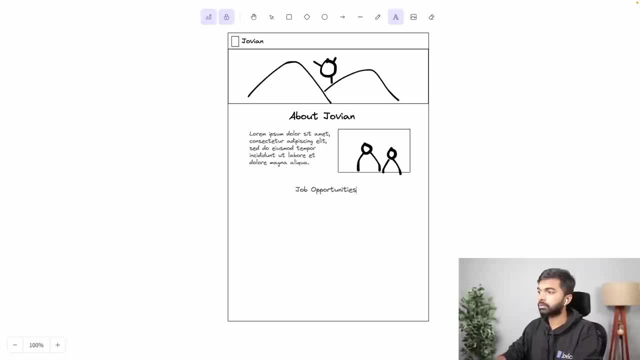 Okay. So let's do that, Okay, Let's do that, Okay. And in this section, job opportunities, I'm going to just make that black in color once again in the section called job opportunities, Let's make that a little bigger, like that. 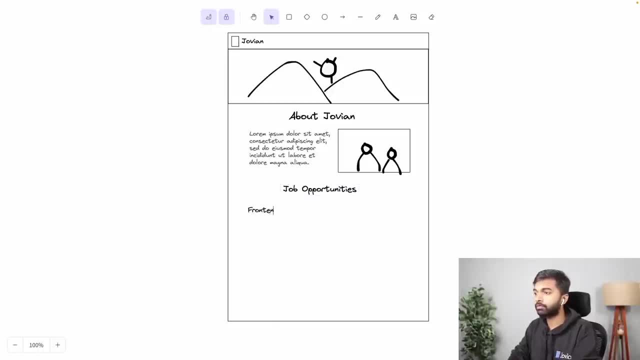 Let us put in a few job roles. So we have a job role for a front end developer, and then we have a job role, and this is in Bengaluru, India. Okay, So we have a job role for a front end developer, and this is in Bengaluru, India. 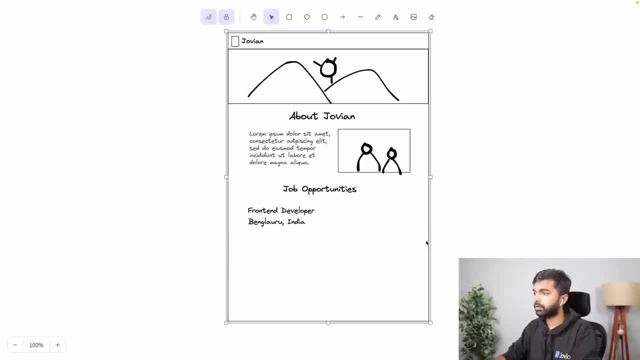 And maybe we want to like an apply button here, or an apply link or apply button or something. Let's put that here. Small apply button. Let's make this a little smaller, like that. So that is what our- uh, that is what a single job role looks like. And now, once again, the good thing about these digital whiteboards is I can use them. So that is what our- uh, that is what a single job role looks like. And now, once again, the good thing about these digital whiteboards is I can use them for a lot of different things. 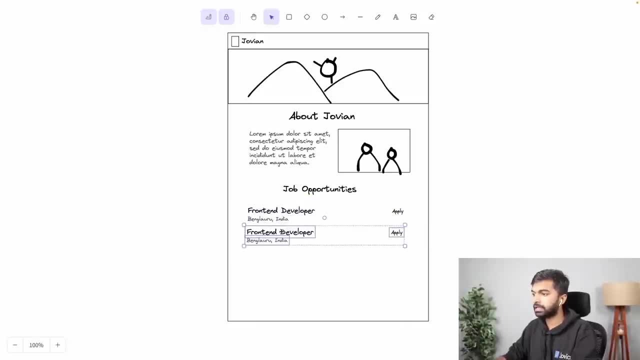 me, I can just take this and I can create a copy and create a second job role and copy and create a third job role. All right, So let's call this backend developer and let's call this data scientist, And maybe let's also put something like remote here. and let me put Mumbai, India, here. 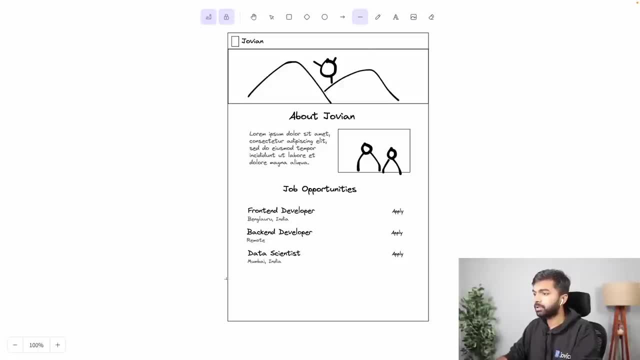 Right, And apart from the jobs, we may be also want to have a footer at the bottom of the page. So I'm going to just add a separation here and maybe I'm just going to add a few links, So one link to courses, one link to programs and one link to YouTube. Okay, And just put that in here. 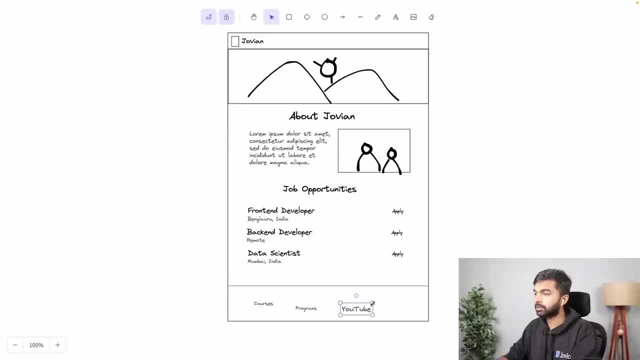 courses, programs, YouTube. let's line these up. So these are going to be our footer links. And finally, right at the bottom, I'm just going to add a copyright notice: copyright 2023.. And let's make that a little smaller and put that in here as well. Okay, 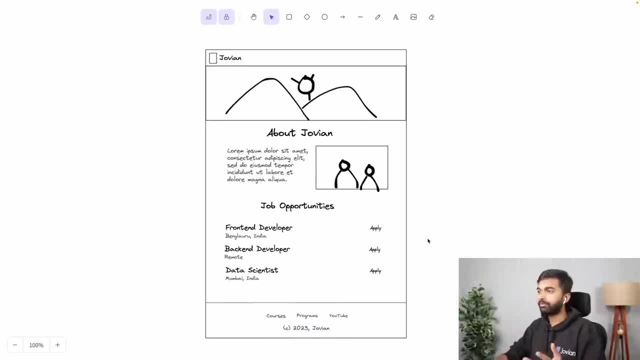 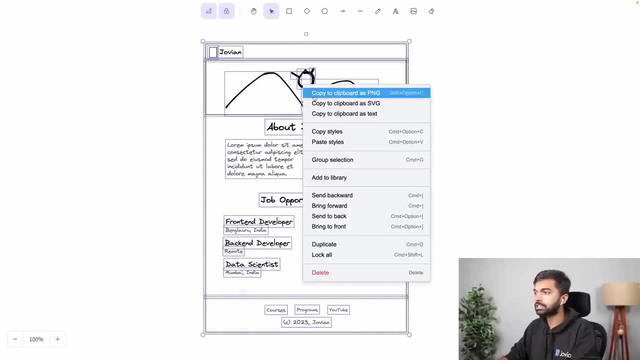 So yeah, just in about four or five minutes, we have just created a wireframe for what our webpage should look like. All right, And then you can cop. you can take this whole thing and you can copy it as a PNG and save it somewhere. Maybe you can send it. to send it to a coworker for review, You can. 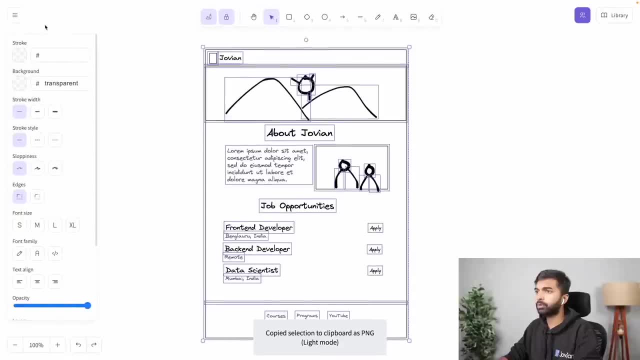 just like copy that as a PNG Or I think you also have the option to export it. You can go in here and you can actually export the image as well. So this is a good thing to do Anytime you're building a webpage. first, it's a good idea to just go ahead and create a wireframe using a digital 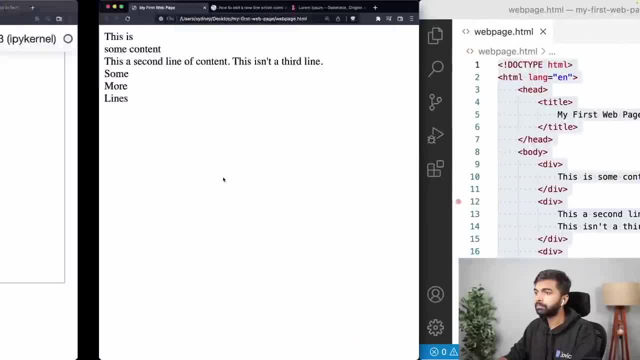 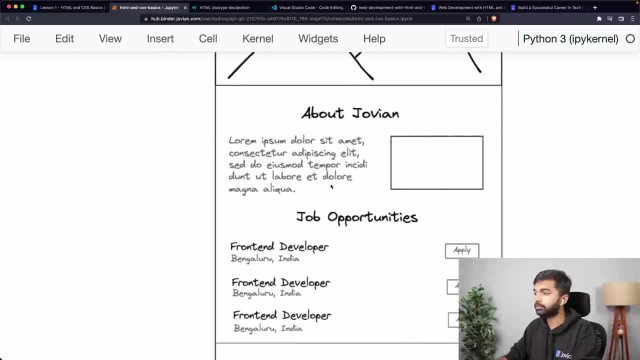 whiteboard and something that you can modify easily as well. Okay, Now that we have this wireframe, you can see here. this is what the wireframe looks like. We have the toolbar, We have an image, We have an about Jovian section. We have the job opportunities. 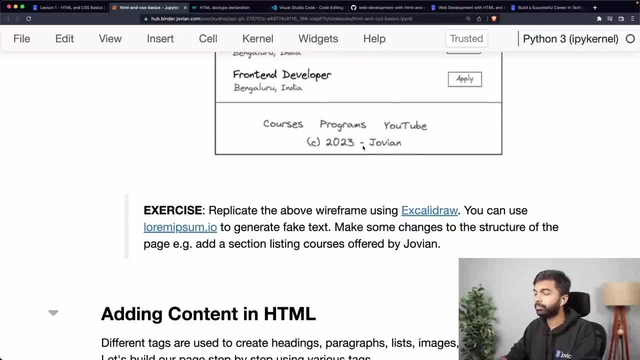 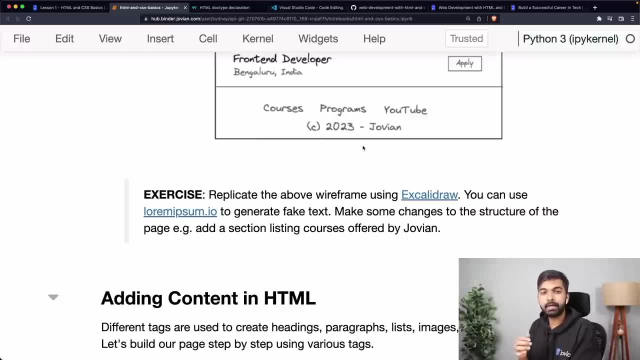 We have an apply button or apply link, and then we have a footer at the bottom. Okay, So I encourage you to again try and replicate this wireframe on your own using Excalibur, or maybe try adding a additional section here and there, just to see if you can do this on. 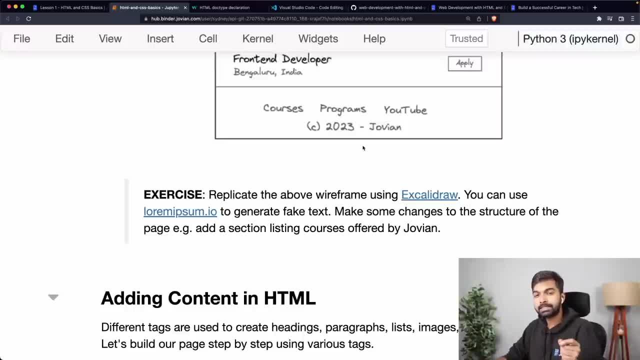 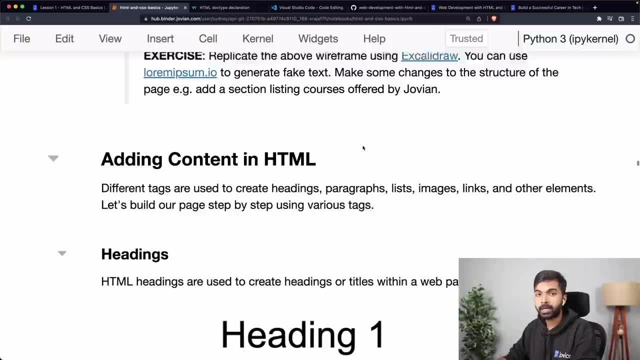 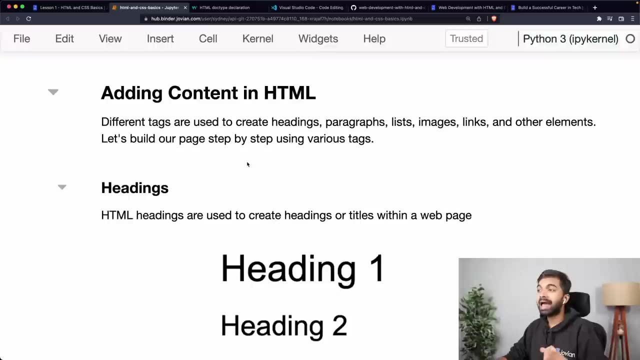 your own. Okay, So you should be following along with this lesson, pausing the video, following along, pausing the video, following along and trying to make changes here and there, just to experiment with things, Okay, Okay. So, now that we have created this wireframe, we can now use this wireframe as a reference to 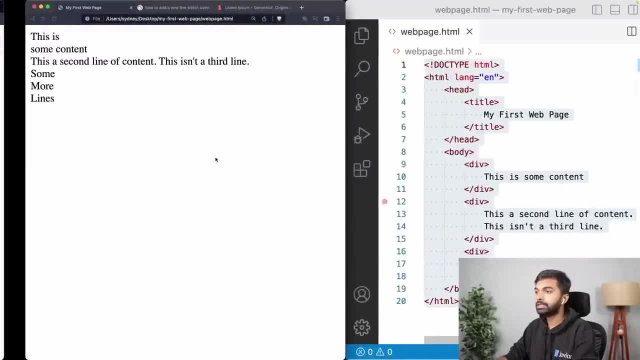 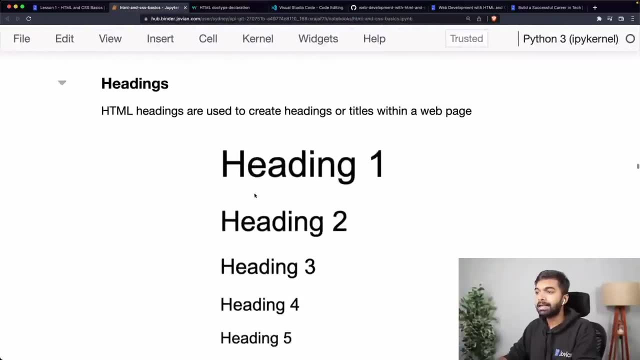 add content in our HTML page. Okay, So right now we don't have any useful content in our HTML page, so we can start adding the content one by one, And the first thing that we're going to add is headings. So let's figure out what headings we have within our webpage. 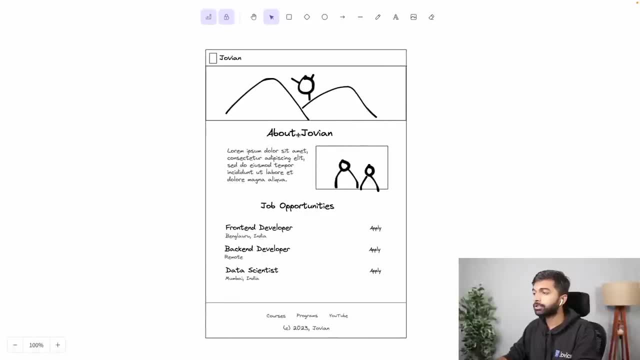 So here we have a couple of headings. We have this heading called about Jovian, We have this heading called job opportunities, and then I could even consider these as headings of each of the different headings. Okay, So let's go ahead and create this. So let's go ahead and create. 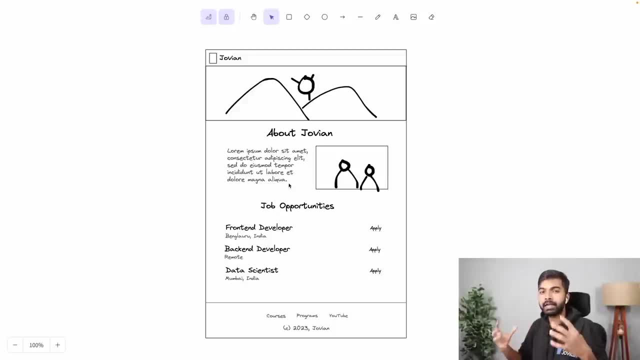 jobs. Okay, So heading is generally just some big text on the page. It is maybe the start of a section, It is maybe a start of a subsection or it is maybe the most important piece of text in a particular element on the page. So I'm going to consider about Jovian job opportunities and front. 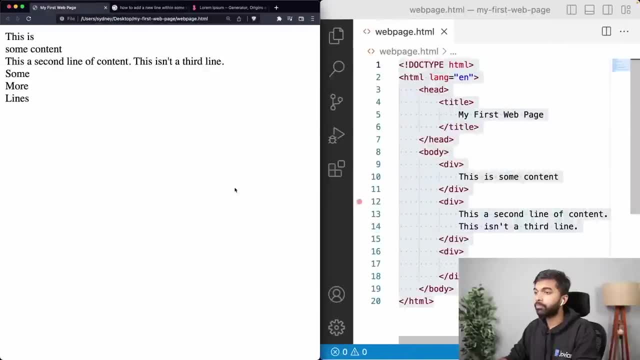 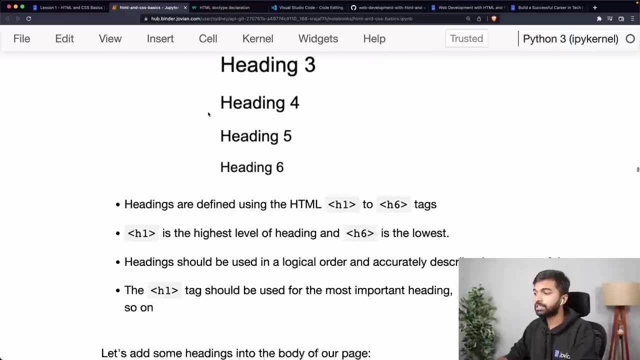 end developer, backend developer, data scientist- as headings. Now, there are various kinds of headings in HTML. In fact, specifically, there are six heading tags. These tags are H1 to H6, and H1 is the highest or the biggest heading. And H1 is the highest or the biggest heading And H1 is the 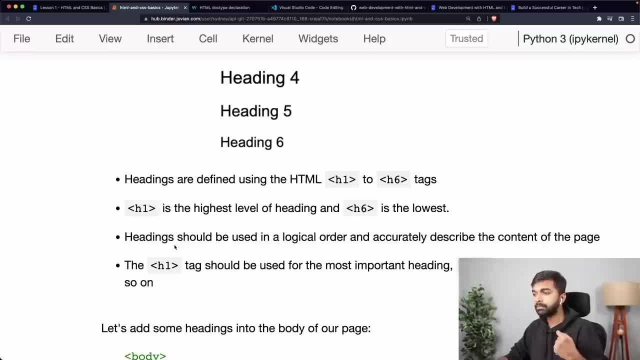 highest or the biggest heading tag and H6 is the lowest. Now heading should always be used in a logical order and should accurately describe the content on the page. So if you're using H1, then for subsections you should be using H2, and then for sub subsection you should be using H3, and so. 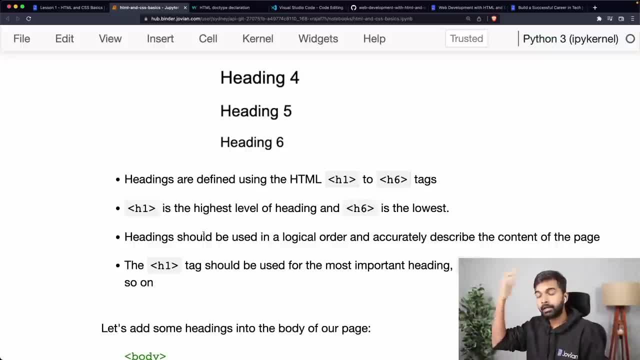 on. Don't use an H2 as the heading of the entire page and an H1 in the middle of the page, because that is going to confuse people, even though you can change their font sizes from the default, but still it's logically it makes sense for you to use. 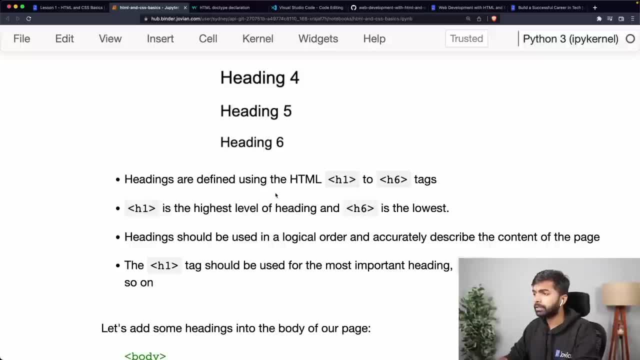 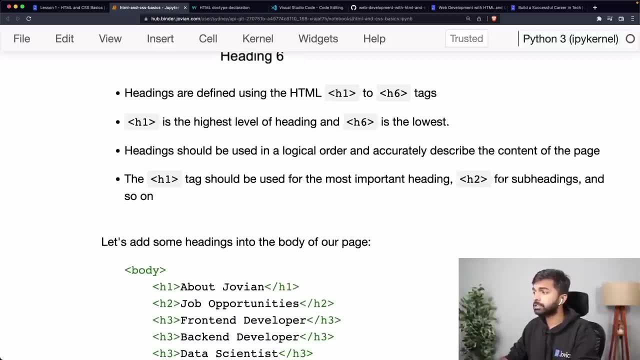 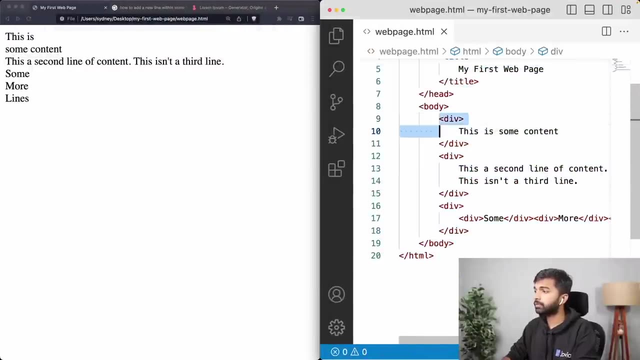 use the headings that are. use headings appropriately within the page. So H1 should be used for the most important heading, H2 for the subheading, and so on. So let's go ahead and let's add some headings into our page. So the first thing I'm going to do is clear all of this. 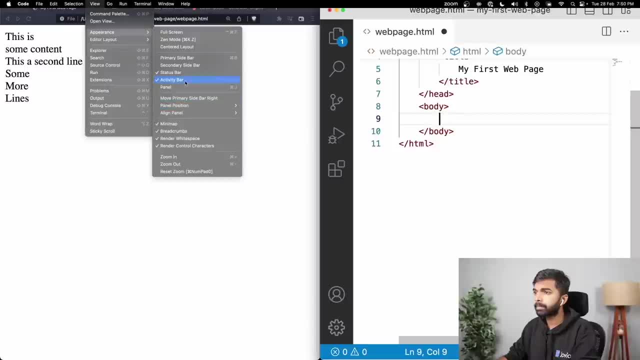 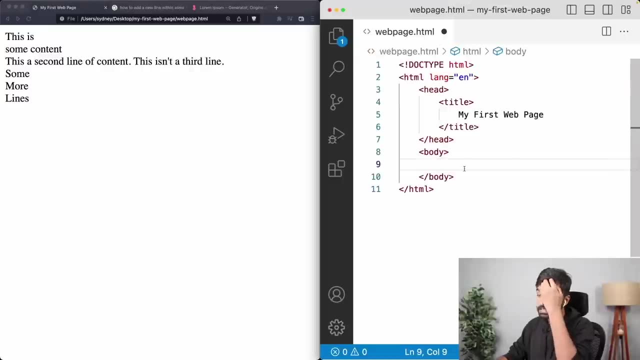 Let me also just, let's see, let me get rid of this piece over here. Yeah, so the first thing I've done is I've cleared out all the existing content on the page And let me save that and that. that is all gone away. Let's add the headings one by one. The biggest heading, 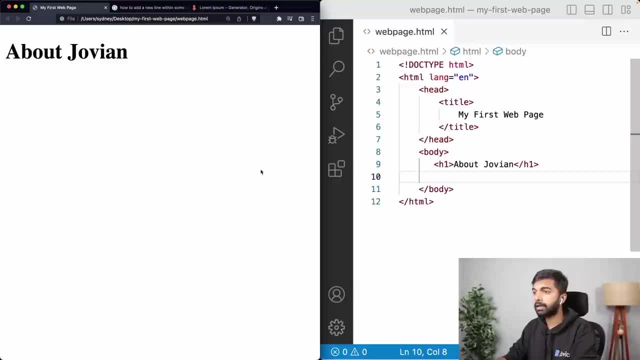 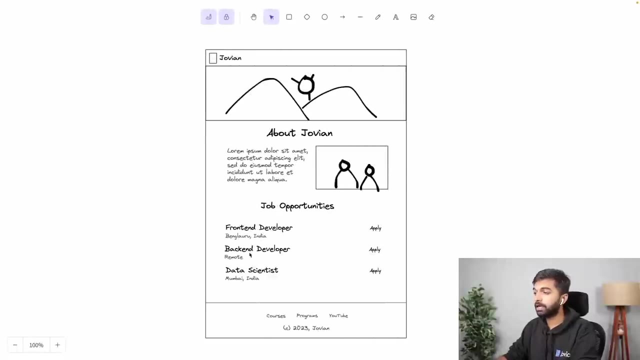 on my page is about Jovian, So let me add that, And once I do that you can see that. okay, now I have a nice big about Jovian section. The next heading on the page is job opportunities- Great. And then we have three of these jobs. So you can see, here we have front end developer. 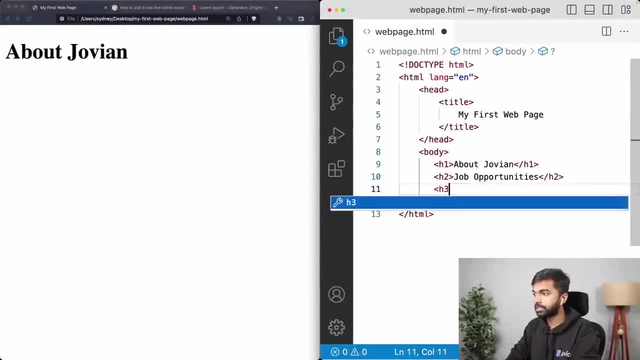 back end developer, data scientist. So let's go: H3- front end developer, H3- back end developer and H3- data scientist. I can go up to H6. But I'm just going to use these three headings here. Now we have this nice. 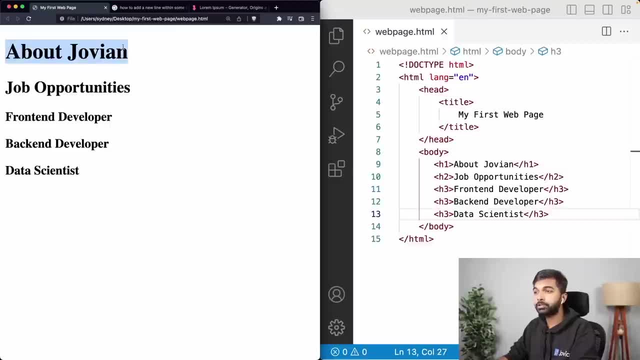 logical separation between headings. So we have about Jovian, then we have job opportunities, And then we have these three job roles, And all these three job roles should use the same header, ideally, because they're indicating the same level of hierarchy. Okay, so that is how you. 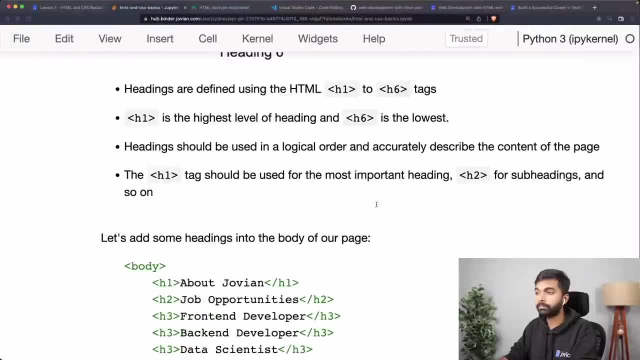 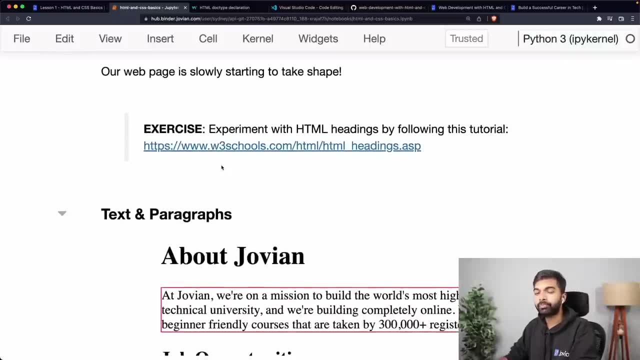 create headings. really straightforward: just put H1,, H2, H3 and keep going. All right, Now we've added headings And this is what that looks like- Great- And our page is starting slowly starting to take shape- Not exactly what we're looking for just yet, But it's getting there. 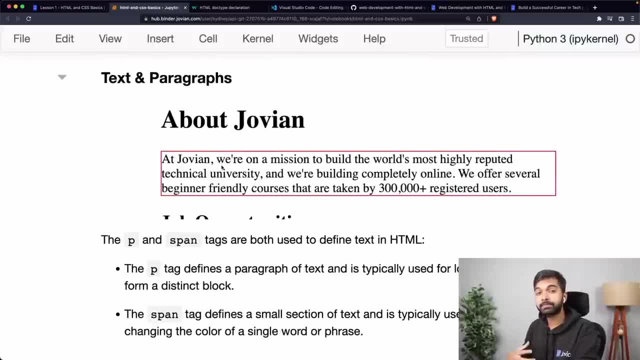 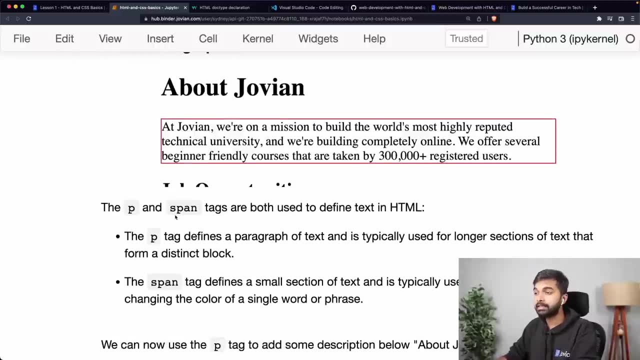 Is there are specific text there's. there are specific tags for adding text. Specifically, we have a couple of tags: One is a p tag or a paragraph tag, And the second is a span tag, And both are used to define text in HTML. So this is some text you can see that we are going to add. 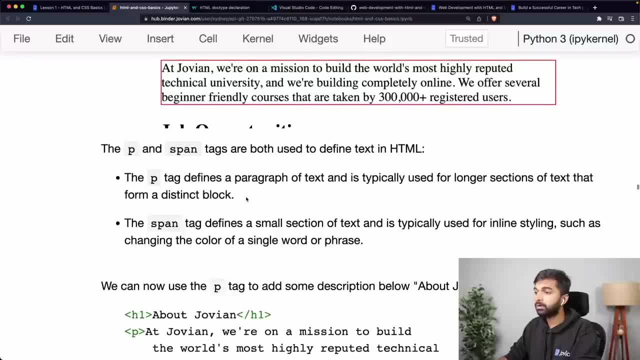 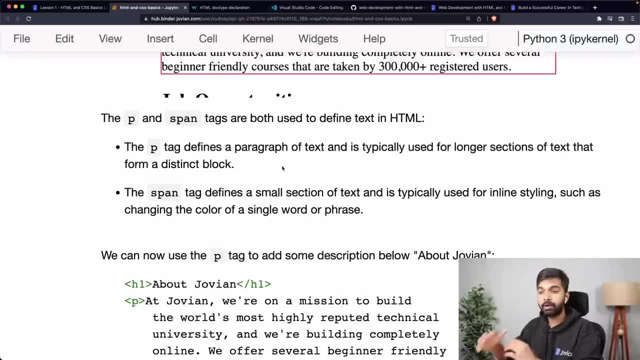 below about Jovian, and this is added using the p tag. So the p tag defines a paragraph of text and it is typically used for longer sections of text that form a distinct block. So if you have an paragraph, that is what you should put into a p tag, And then the span tag defines a small section. 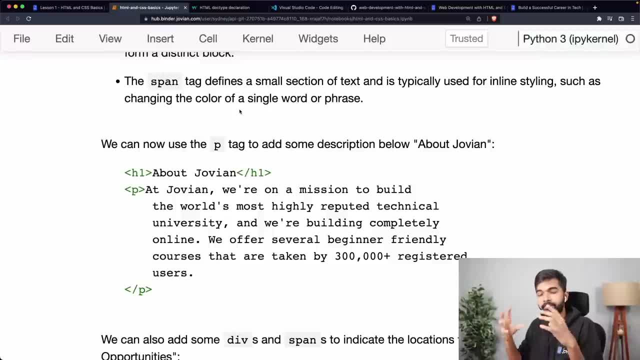 of text. Typically, if you have maybe just a few words or maybe a single line somewhere within a div, you can use it, And it is typically used for inline styling. Let's say, you have a longer piece of text and within it you want to make some specific piece of text bigger or 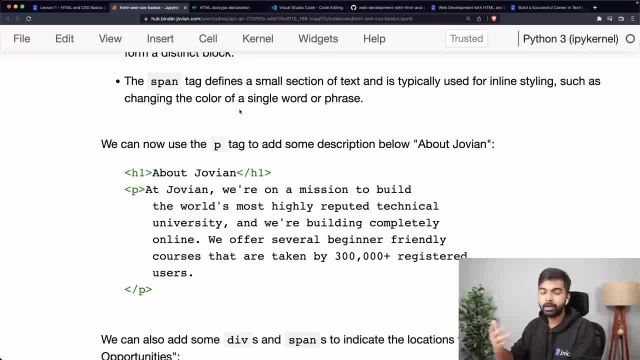 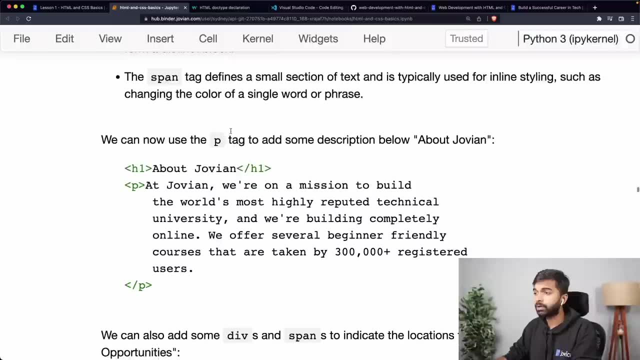 of a different color, then you would wrap that around a span And we look at examples as we go along. But p and span are the two tags that are used to create text on a web page. Of course, you don't need to use a span or a p. you can directly put a text within the div. 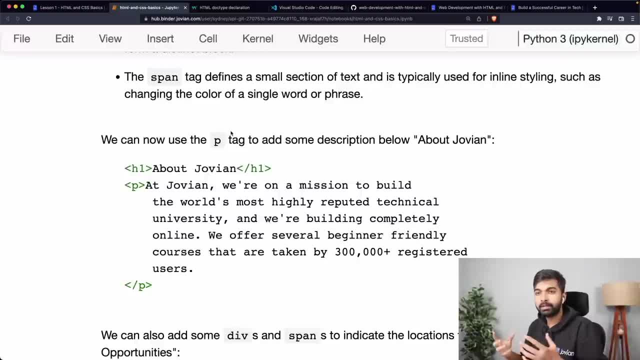 tag, as you saw already. But p and span give some one. they semantically inform the browser that now inside this tag there is going to be text And second, the div is going to automatically create a vertical separation. The span doesn't do that, So sometimes if you want text to maybe join. 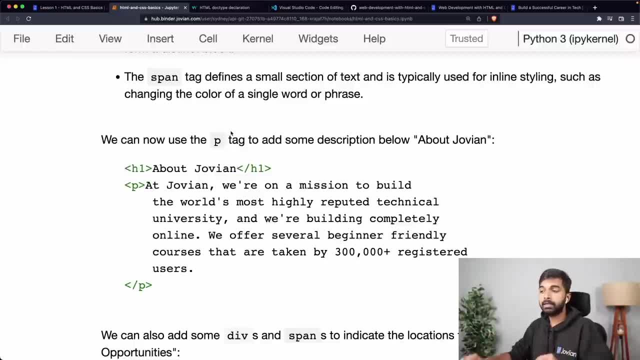 together and show up in a single line. you can use a span And the p tag has some spacing before and after, So it automatically adds some separation. The p tag is the one that creates some between the text and the rest of the content. Okay, So let's use the P tag to add some description. 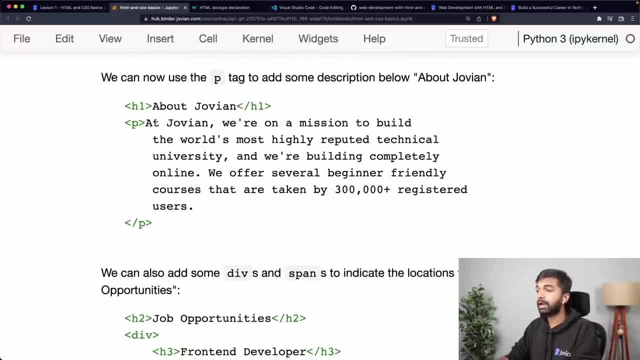 below about Jovian. So here is the description that we're going to add: at Jovian, We're on a mission to build the world's highly, most highly reputed technical university and we're building it complete, building it completely online- Let me change that to it- And we're 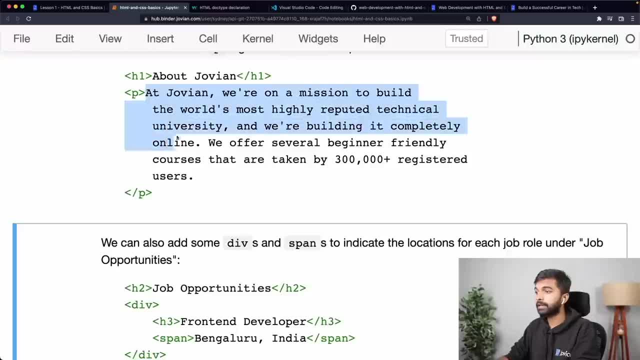 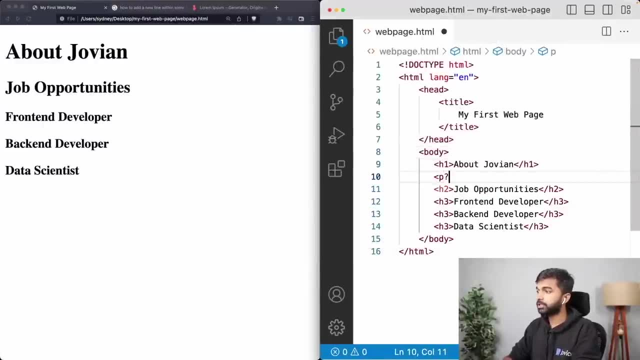 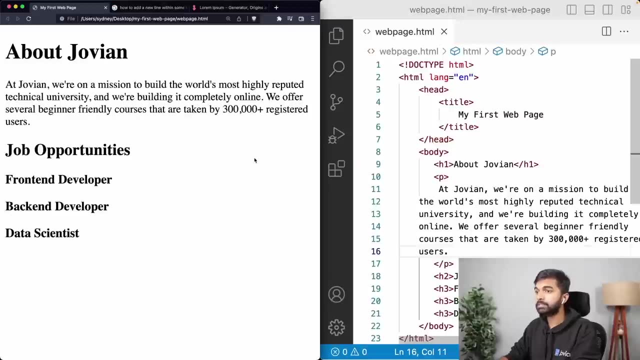 building it completely online. We offer several beginner friendly courses that are taken by 300,000 plus registered users. Okay, so, right below the H1, right below the section here, I can put in all of this content And I can just click Save And then I reload this And. 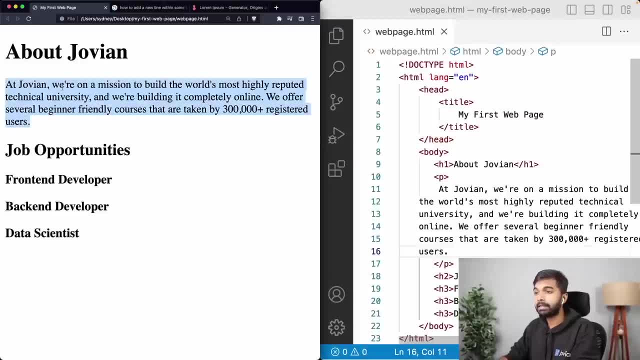 you can see that this P tag has been added And in this P tag we have this basic text. Now somebody had a question: why not use a div tag here? Well, if I just use a div tag, you can see that the amount of 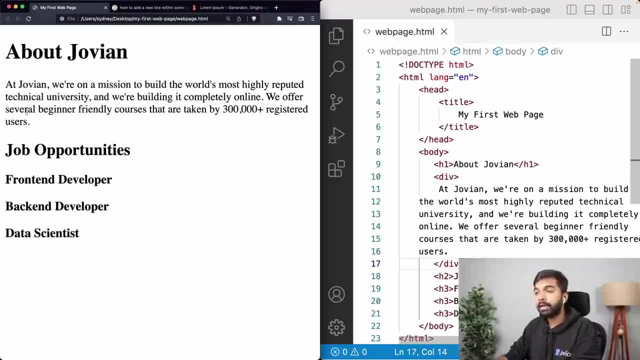 Well, it works just just just fine. But, as you noticed, as we put in multiple paragraphs of text, you will notice that the P tag automatically add some gap between paragraphs. So that is going to be the difference between using a P tag versus using a dev tag. 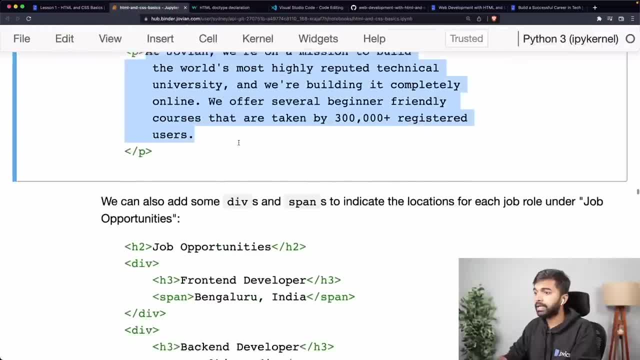 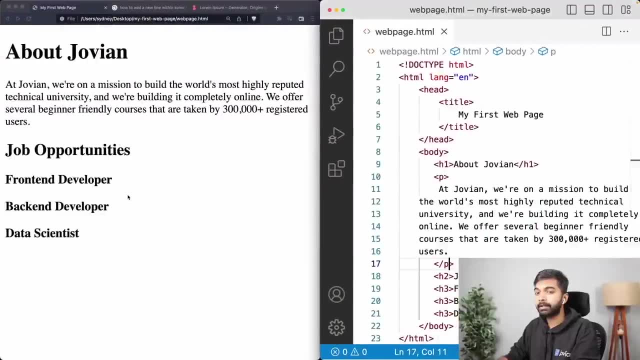 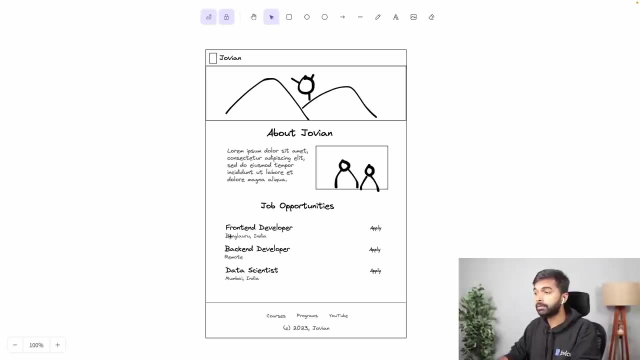 All right, So now we've added a P tag. Then the other place where we can possibly use a span is within the job opportunity section. Notice that under each job opportunity we have also put in the location of the job. So let's put that location of a job using. 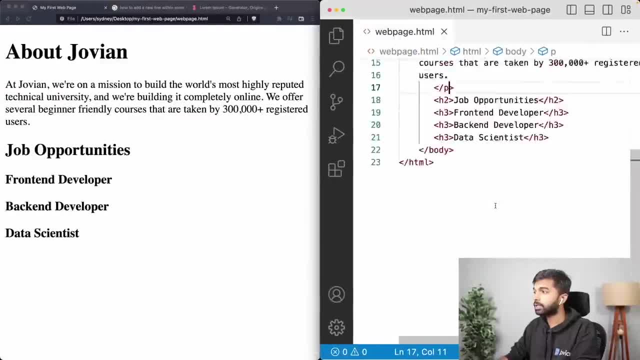 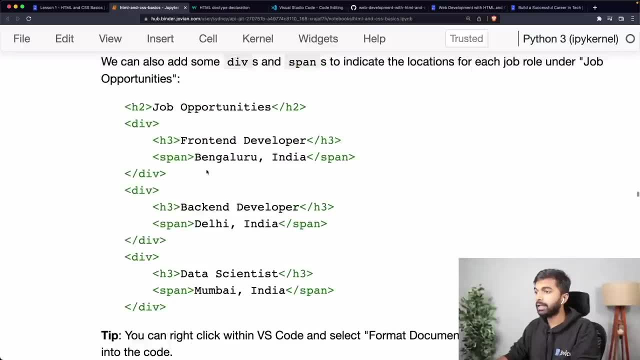 the using a span. Okay, so here's what I'm going to do. I am going to first wrap, I'm going to create a span And I'm going to take the span and the h3 and put that in a div tag, Because each job is logically separated, So each job we wanted to show up in a logically 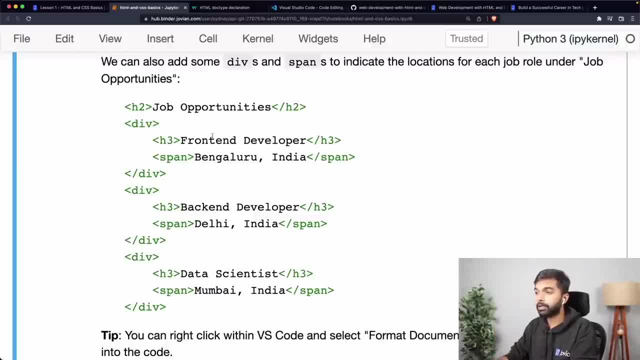 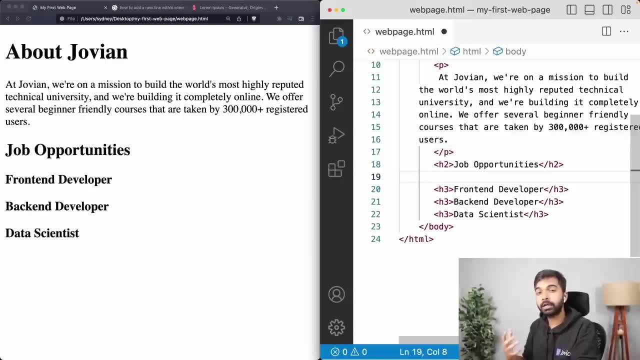 separated area. That is why we're putting a div around the job. Okay, And don't worry if this doesn't make sense. If you're wondering when should I put a div around something, when should I not put a div around something, Well, you just experiment with it. Extreme html is all about experimentation. 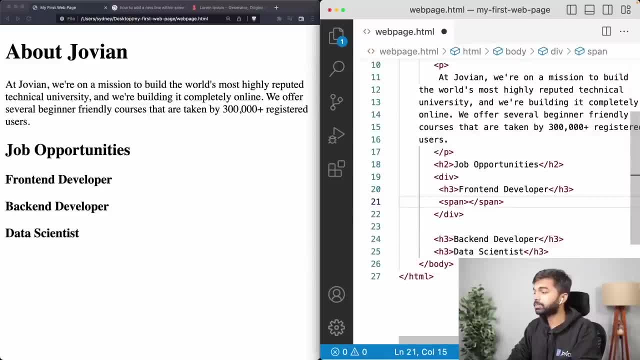 Right, So here we have an h3 tag and then I'm going to put a span and I'm going to put in Bengaluru, India. Then I'm going to put in another div here And I'm going to move this back end developer role here and I'm going to put in a span, I'm going to put in 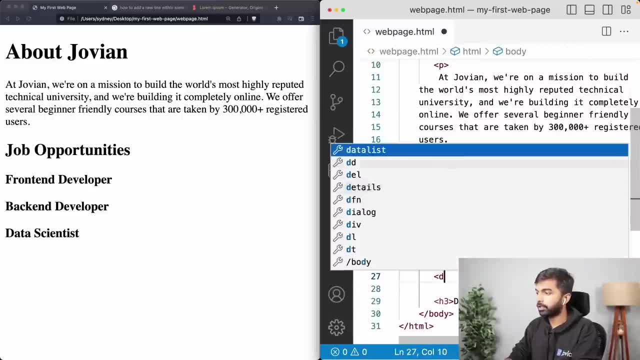 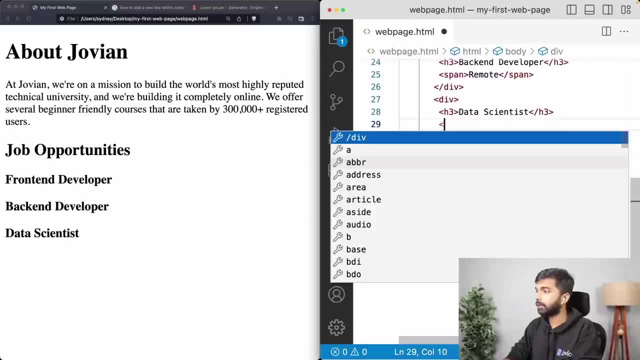 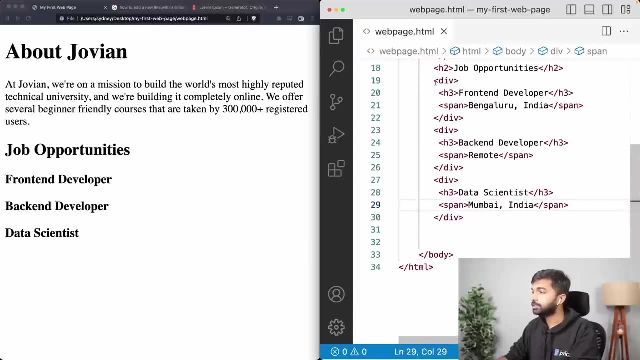 let's put remote here, And I'm going to put in another div here And I'm going to put in the third h3 here And I'm going to put in a span. Let's put Mumbai, India, here. Okay, so now we have added these job opportunities locations and we put each of the 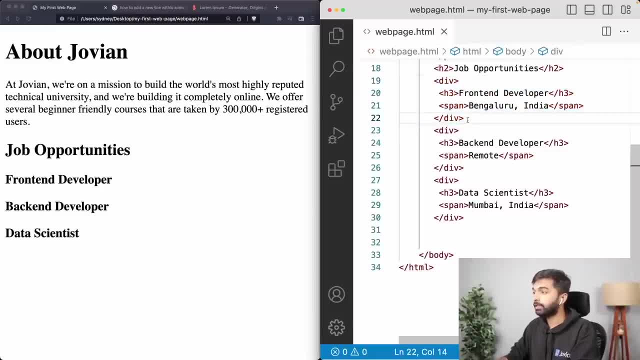 job opportunities plus location in a div tag. Now one quick thing I want to show you is: let's say you're typing and maybe things go a little bit haywire And you don't have this nice indentation or this nice logical structure visible anymore. just right click and select format document. 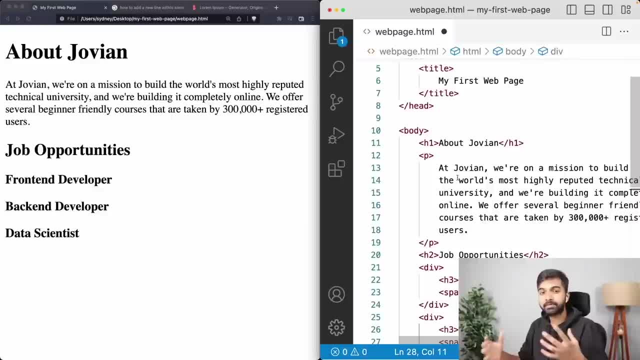 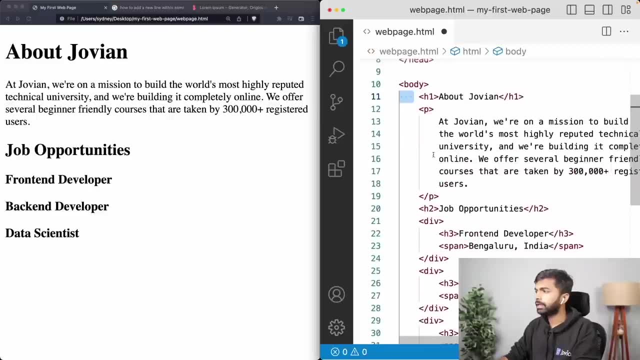 And that is going to automatically arrange all the tags in this nice fashion that tags that are children of an outer tag are automatically going to get some indentation or some space before them, And then it's also going to split up the lines nicely. So anytime you want you can right click. 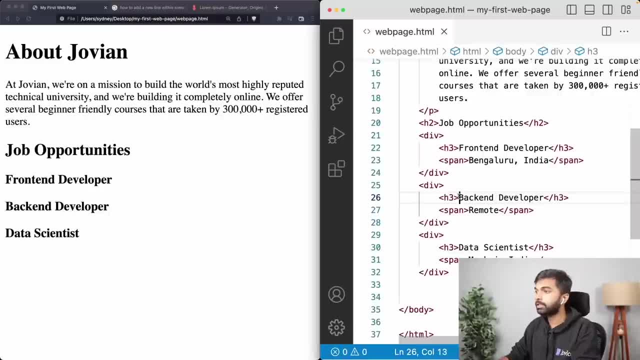 and select format document, And there's also a keyboard shortcut to do it, and then you can save it And let's reload now And alright. so now it's starting to look a little better. Now we have the front end developer role And under it we have Bengaluru, India. 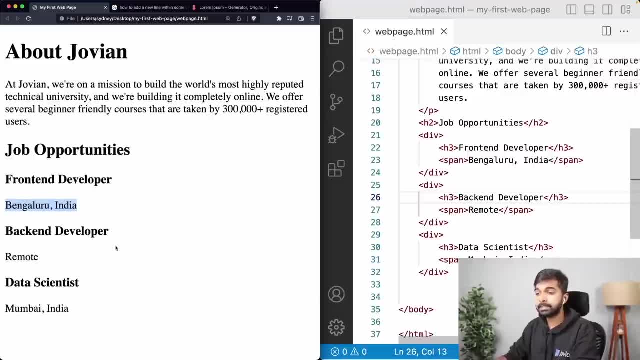 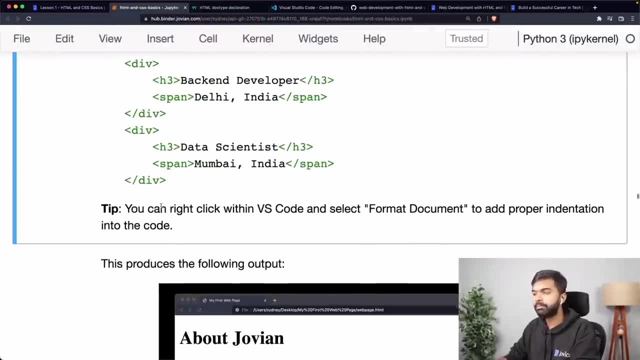 then we have back end developer under it, we have remote and data scientists under it, we have Mumbai, right. So our notebook, our web page, is starting to take shape pretty nicely, Okay, so now we have this information Now. apart from this, there are also several. 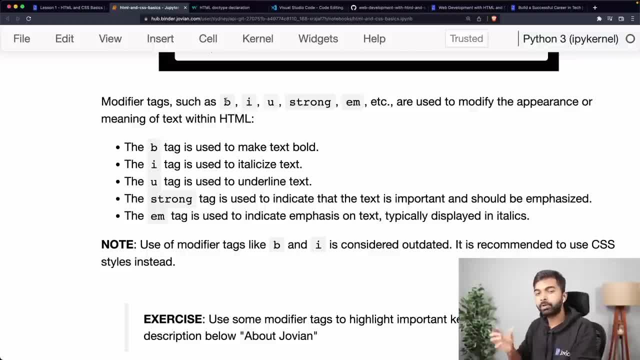 smaller modifier tags. So there's a tag called B in case you want to make something bold in within a paragraph. There's a tag called I in case you want to make something italic. There is a tag called you in case you want to underline something. 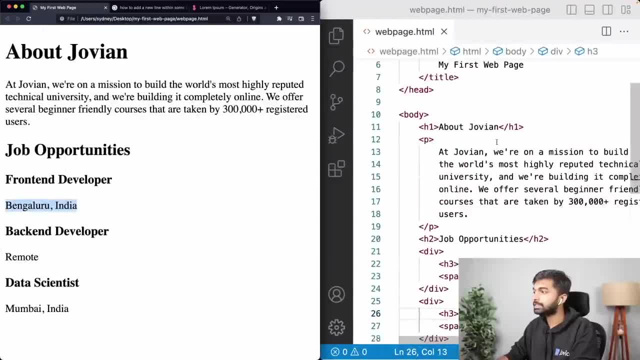 Now you can use these tags in between. I'll show you an example. let's say we want to highlight 300,000.. Plus, I'm just going to put it in a B tag. So there's an opening B tag. 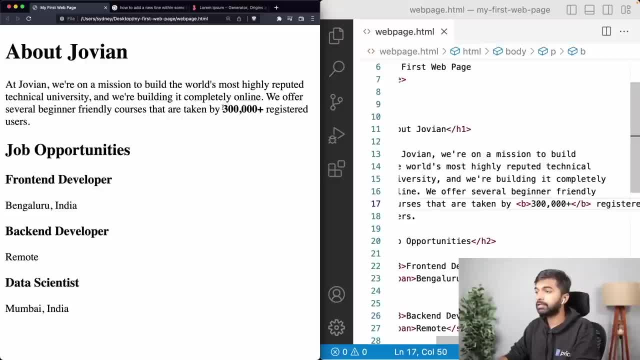 and then there is a closing B tag, And you can see that 300,000 is now bold. However, these specific tags are slowly falling out of fashion. What is being done instead is you just put a span around a specific piece of text and then use it. use. 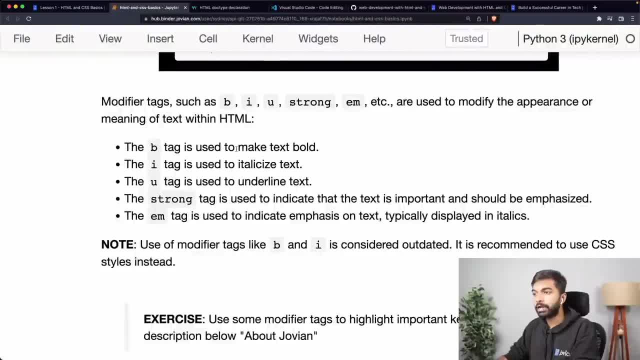 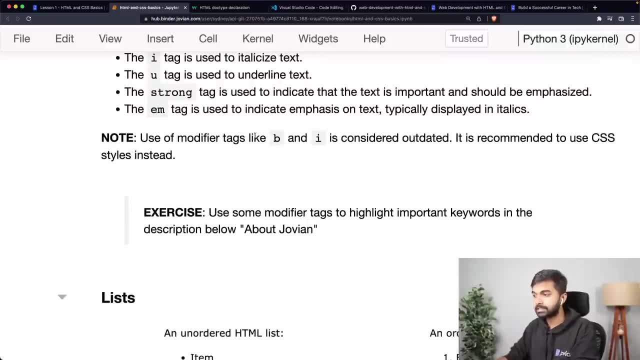 style it, and we look at CSS soon. So just know that, although you have all these tags, the use of these modified tags is now considered a bit outdated and it is recommended to use CSS styles instead. But still, as an exercise, I will encourage you to just play around with these. 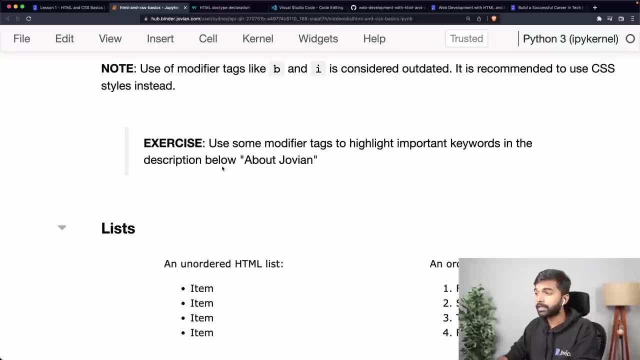 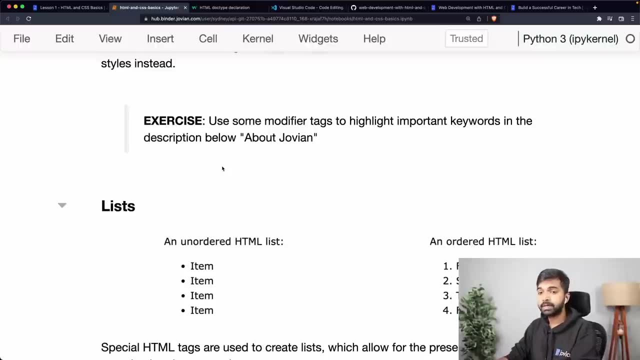 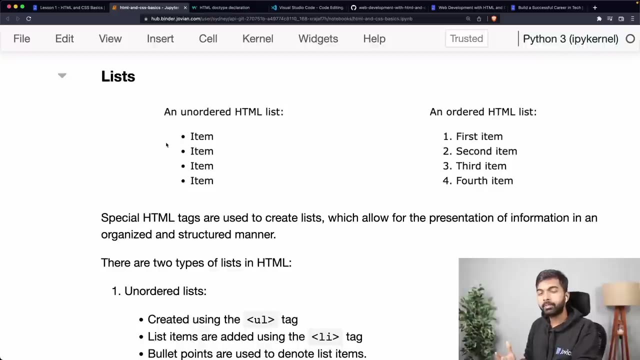 tags and check them out. Okay, perfect. So now we have looked at text, we have looked at headings, we have looked at spans as well. Next, let us look at lists in HTML. So almost every web page that you might have seen contains some form of lists. 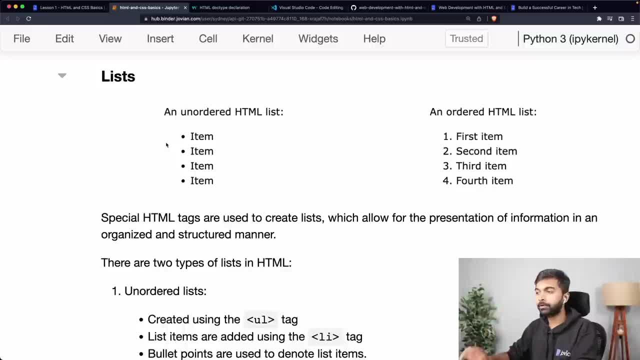 And there are two types of lists in HTML specifically. there are more, but these are the two that are commonly used. One is an unordered HTML list, And an unordered HTML list is simply a bullet list. It does not have any ordering. it is ordered but it doesn't. 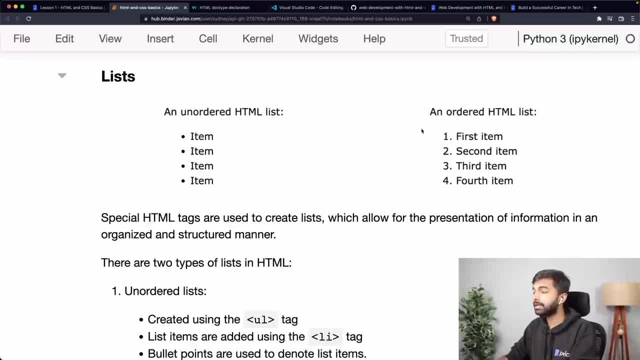 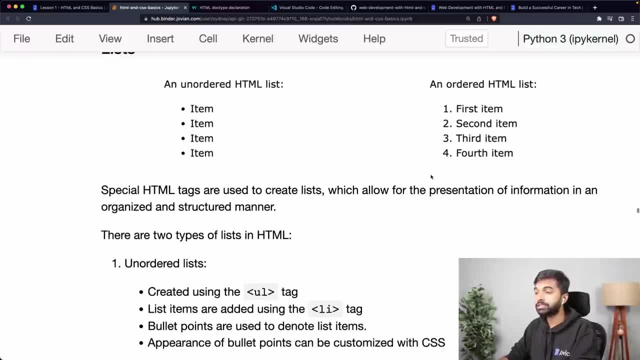 have numbers for the elements or the items within the list, And then you have an ordered HTML list. an ordered HTML list simply has numbers associated with each of the items, And special tags are used to create lists which allow for presentation of information in an organized and. 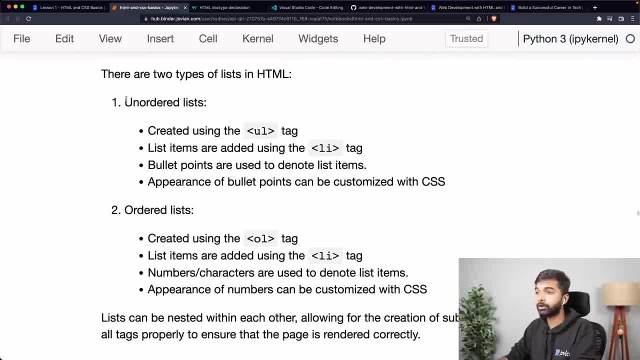 structured manner. So there are two types of lists, as I said, unordered. and the unordered lists are created using the ul tag And then list items within an unordered list are created using the li tag, And bullet points are used to denote the list items And you can change the appearance of bullet. 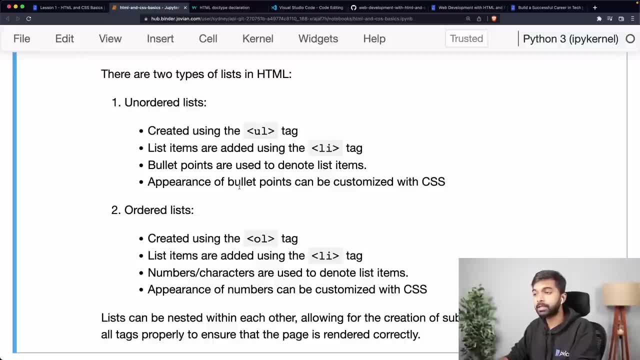 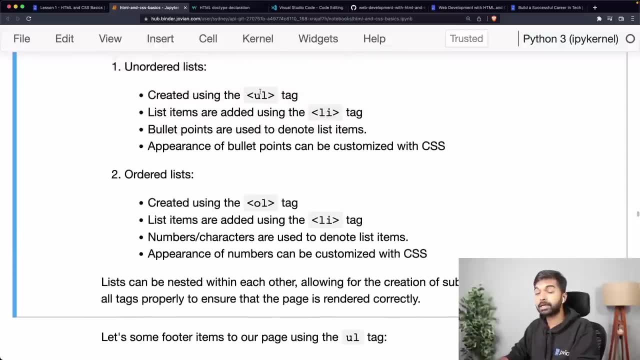 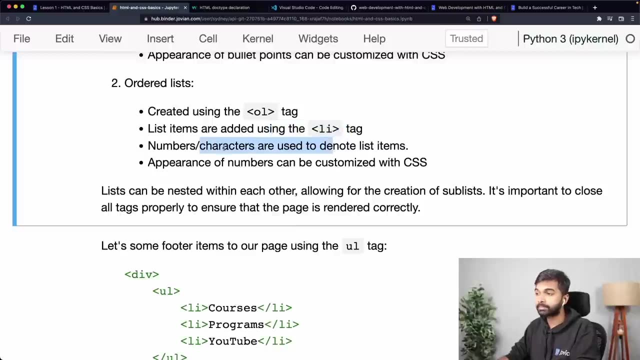 points using CSS or using some attributes as well. Similarly, you have ordered lists and ordered lists using the ul tag, So ol is ordered list, ul is unordered list And list items are added using the li tag, And numbers or characters are used to denote list items And the appearance of the 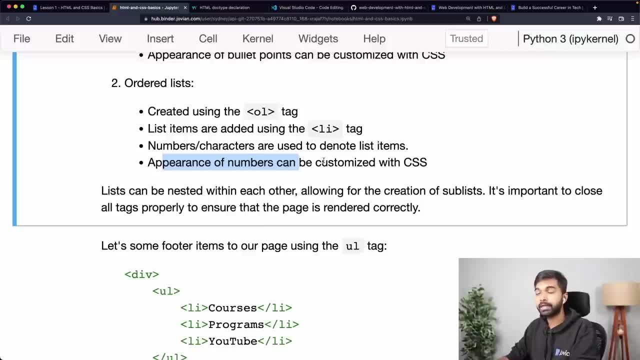 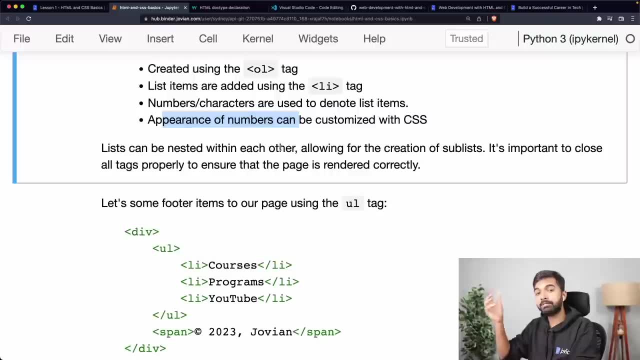 numbers can be customized using CSS or using attributes within the HTML element itself. You can also nest lists within each other, So you can have, maybe, a list, and then each list item can have a sub list inside it, and so on. So you can do a bunch of interesting things, But it's important. 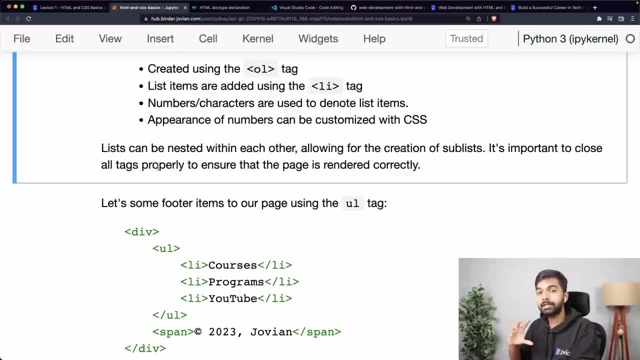 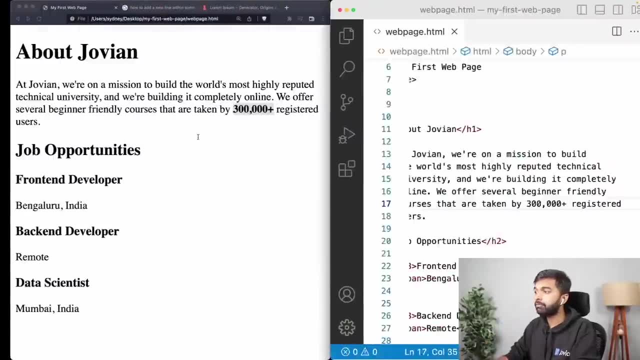 to close all your tags properly Is rendered properly. Otherwise the browser is going to run into issues and things are going to look a little weird. Okay, So remember we had a footer on our page. Let's try, and maybe this looks like a list of links. So let's try and maybe create. 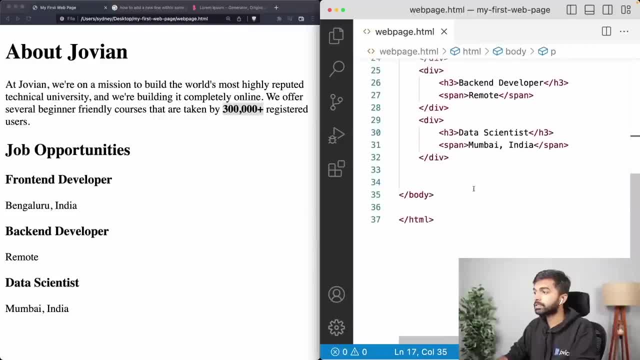 an unordered list for the footer elements. So I'm going to come in here And again, I'm going to just create a logical separation by creating a div And I'm going to create a ul or unordered list, And then in the unordered list I'm going to have three list items. 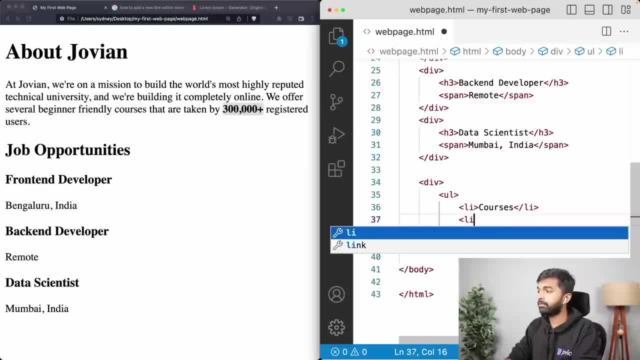 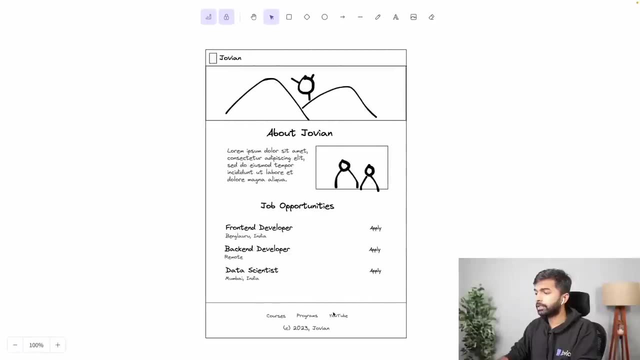 So I have a list item called courses, And I have a list item called programs, And I have a list item called YouTube, And then below this, I also have this copyright thing. You can see, we have this thing copyright 2023, Jovian. So I need the copyright character. 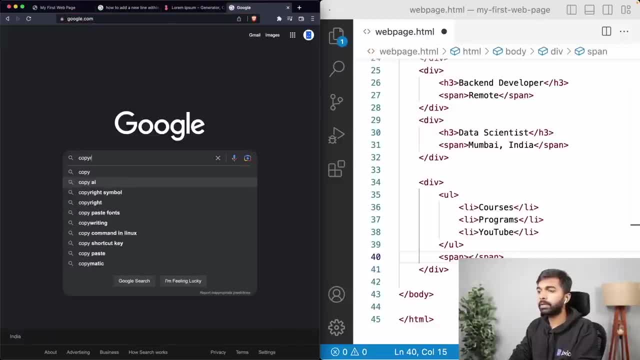 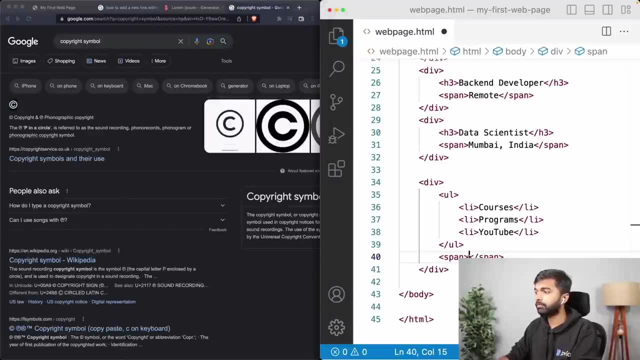 So I'm just going to go on Google And I'm just going to search copyright symbol. Okay, this is the copyright symbol and I can just go Go ahead and copy it from here and paste it. So this is how you get special characters in your 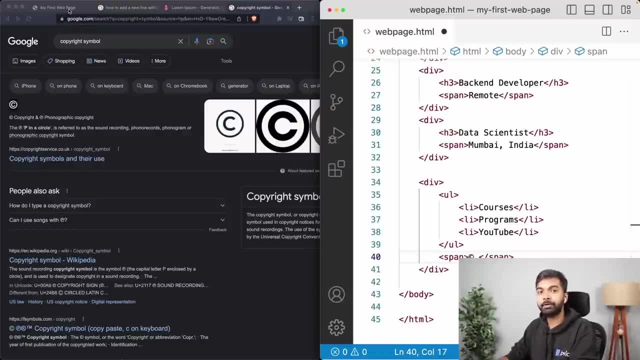 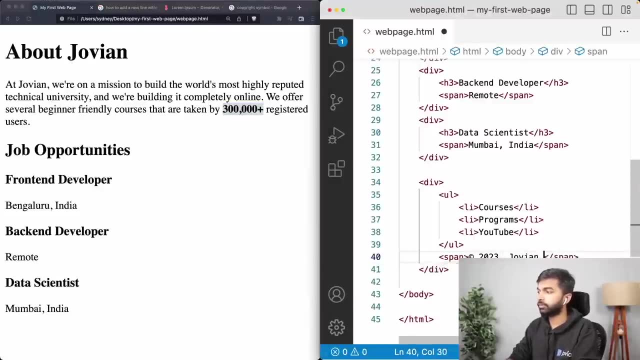 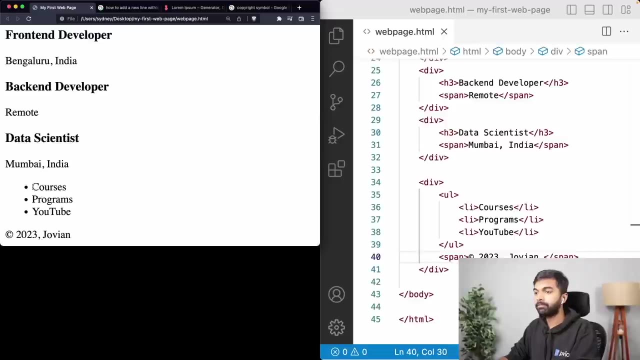 HTML. you just search the special character online and then you can copy it from there and put it in the copyright 2023 Jovian. Okay, now let's reload the page And just like that, you can see here at the bottom of the page we have courses, programs, YouTube. 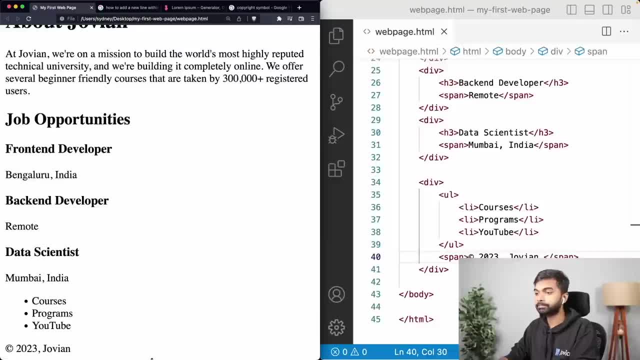 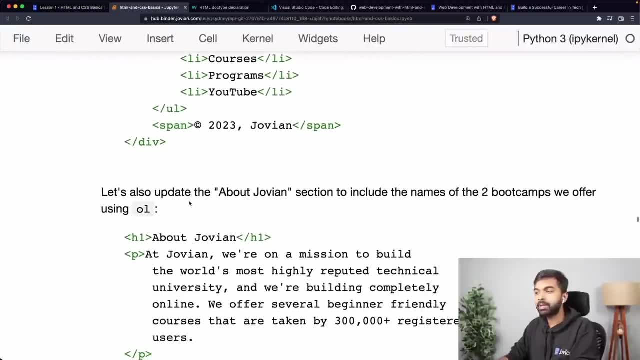 and we have copyright 2023 Jovian Great. So our page is taking shape. Apart from this, let's also add an ordered list somewhere. So maybe in the about Jovian section in this region, let's maybe also list the programs that we offer. So let's add another paragraph here. 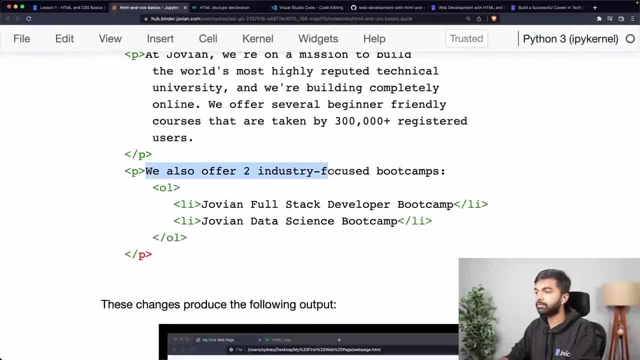 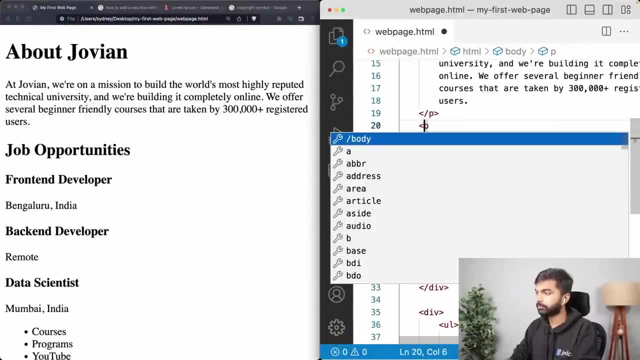 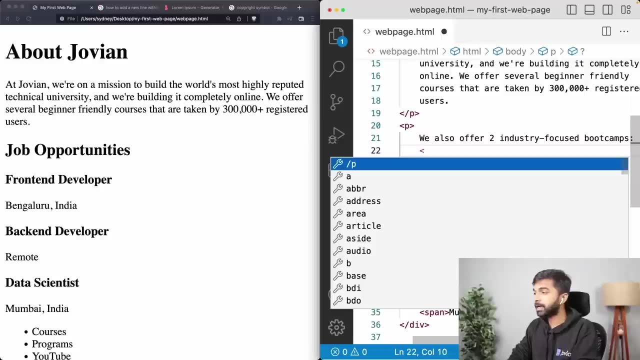 Let's see what we want to do. Well, we add another paragraph and we're going to say: we also offer two industry focused boot camps. So let's create another paragraph P, And let us put in this text: we also offer two industry focused boot camps. And in this paragraph, 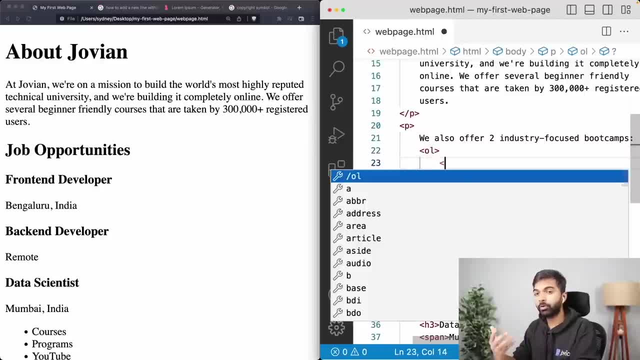 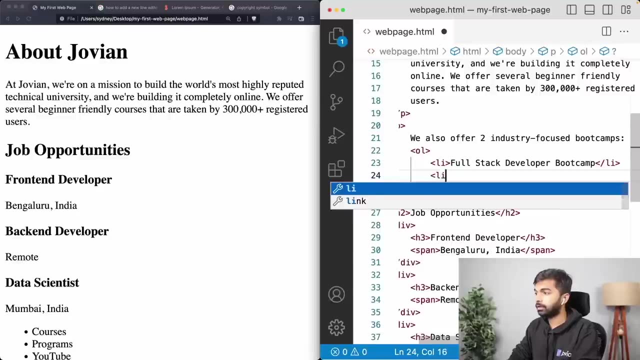 let's create an ordered list, Because we are. we have two programs and we can list them one by one, So let's create an ally here: One- or actually I don't need to put the number one. the number one is going to come automatically: full stack developer boot camp, And then the second one is: 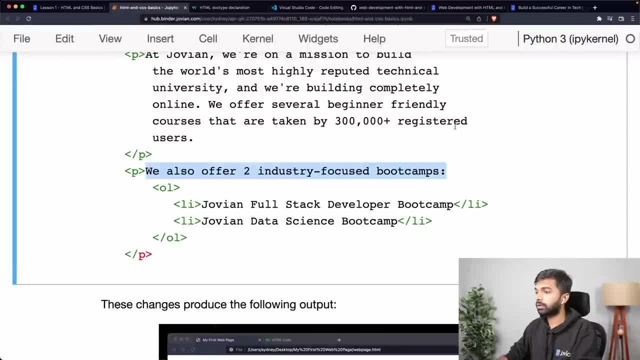 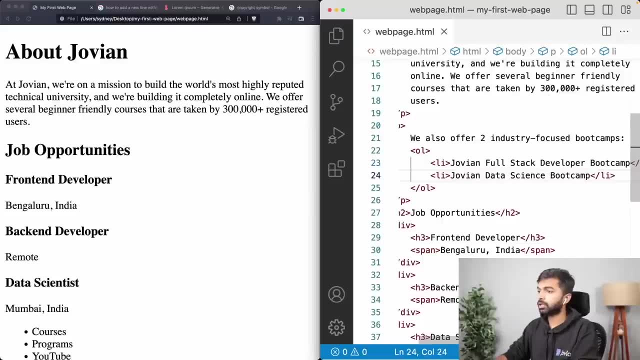 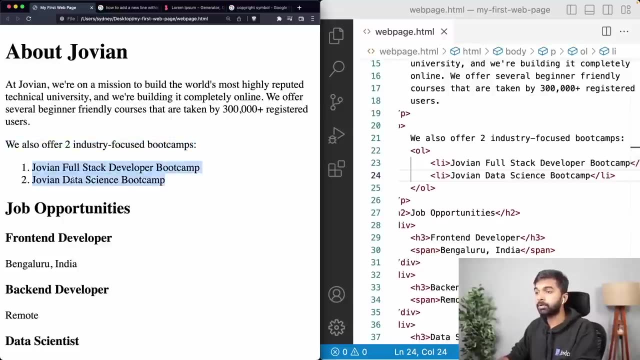 data science: Okay, Okay, I think we want Jovian full stack developer boot camp- Data science. All right, So now you can see that we have. we offer two industry focused boot camps: the Jovian full stack developer boot camp and the Jovian data science boot camp, and the numbers one. 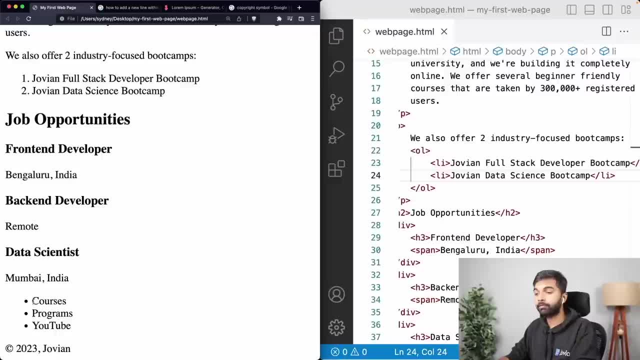 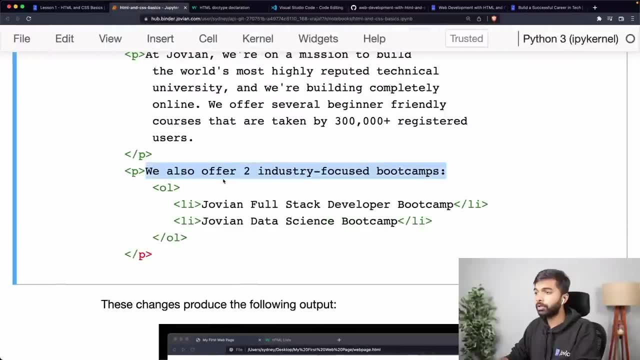 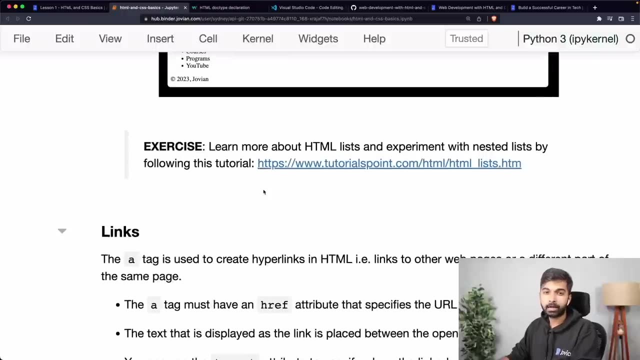 and two have been added automatically, just as it was done in the case of the footer. items were here just added a bunch of bullet points, Great, So so far, so good. We have added some lists as well, And that has added some more content. on the page Next up, we can add some links. Now 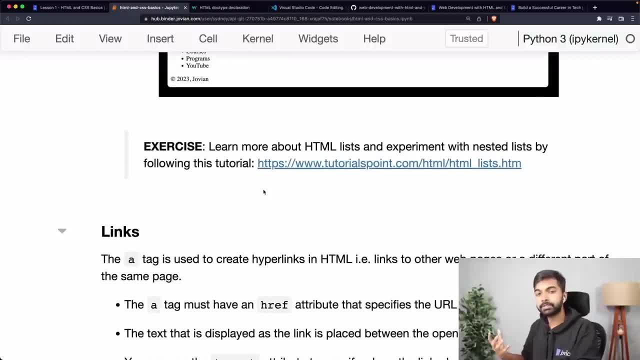 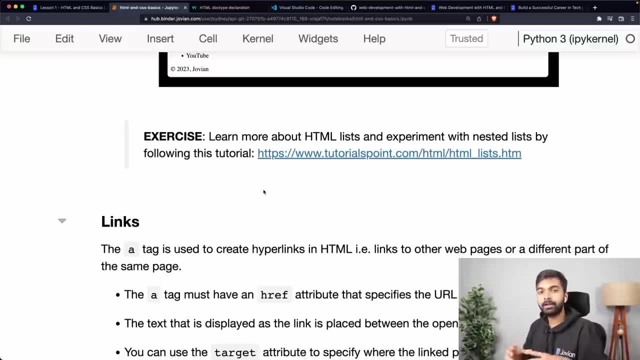 since we have added some footer. we are added some footer items. we also added maybe a couple of programs, So we can now link these two other pages. you know that any web page on the internet typically contains links to other pages, And that is how you navigate a website. Now links can be to the same website. links can: 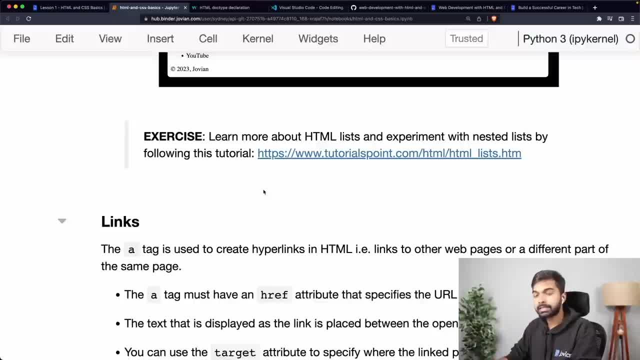 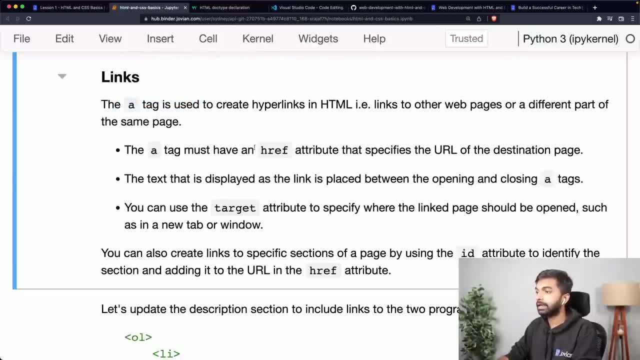 be to other web pages on the internet. it is completely up to you, But links in HTML are created using the a tag. the a tag is used to create hyperlinks And the a tag must have an a tag that is used to specify the URL of the destination page And the text that is displayed. 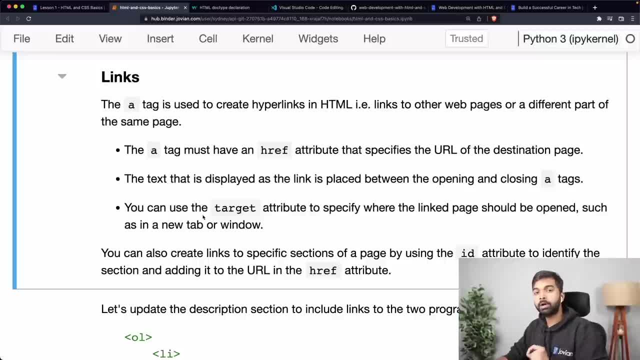 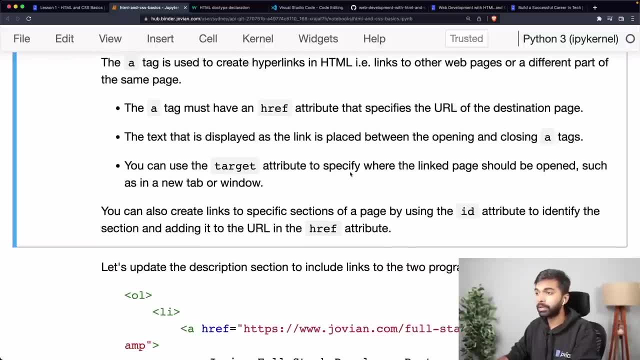 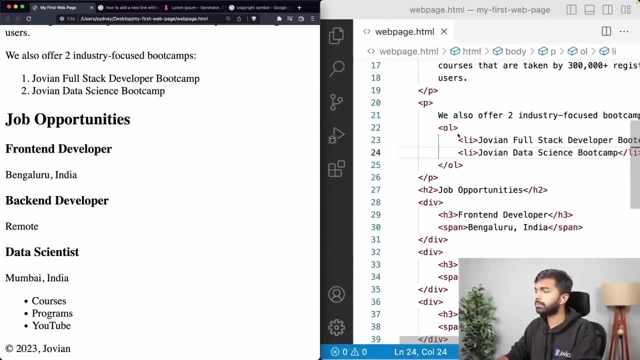 as the link is placed between the opening and closing a tags And let's say you want to link to open in a new tab, then you can use a target attribute to specify where the link page should open. Okay, let's see that step by step. Let's first do this for the Jovian full stack developer. 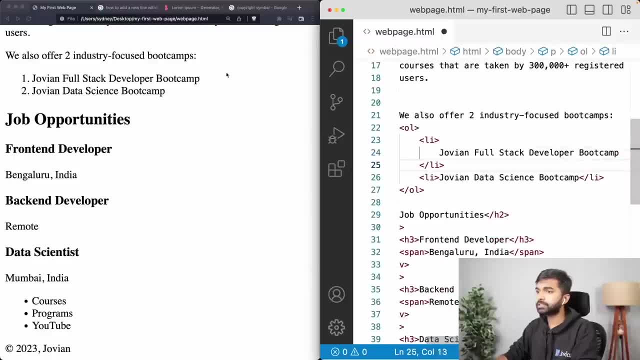 boot camp. So what we, what we want to do is we don't just want to show this text: Jovian full stack developer boot camp. we actually wanted to point to the program application page because, let's say, somebody is applying for a job, But they also want to see what kind of programs we offer. 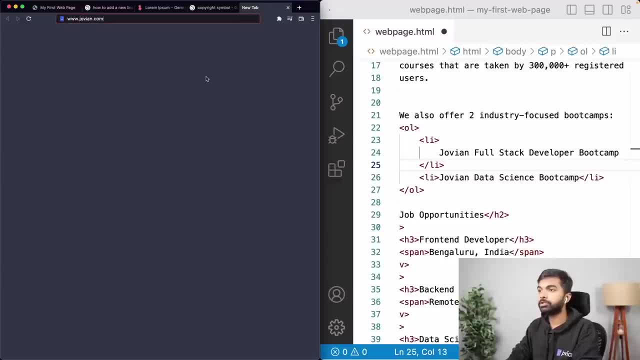 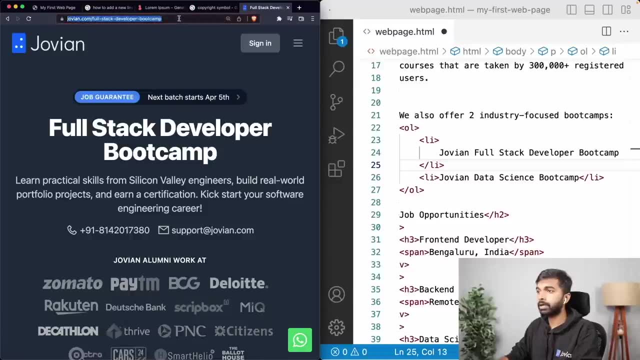 it would be a good idea to maybe just link that from here. Let me go to wwwjoviancom And I'm going to scroll down here and I'm going to find the section full stack developer boot camp and I'm going to grab the link of that And let's come back here And let's create an, a tag inside. 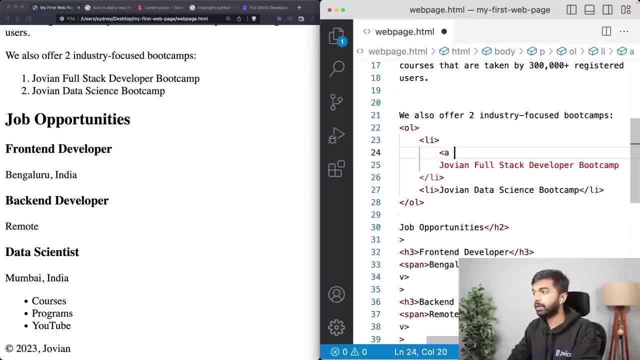 the li item. So inside the list item we're creating an, a tag. so a tag, we're creating an href- hr e f. hr e f is the attribute, And then the attribute value is always put within double quotes. So within these double quotes I'm going to paste the link. 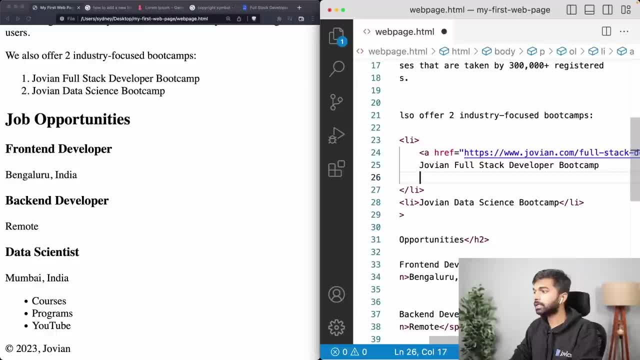 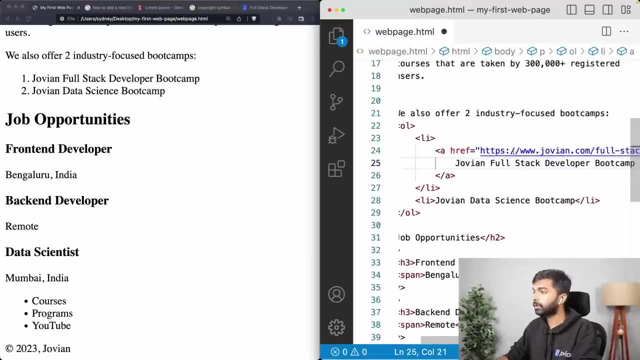 okay, and then I'm going to close the a tag And I'm going to take the closing tag and put it outside the text. Okay, so now you have a href and then you have the href of the other. you have the URL of the Jovian full stack developer boot camp And then you're closing the a tag inside. 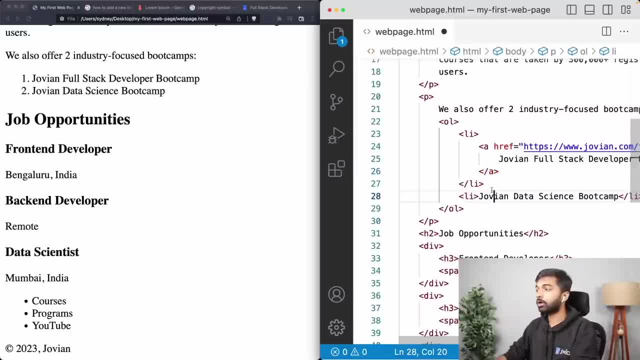 the LI tag. So remember, your tags have to be matched up properly when you you cannot put the a tag- closing a tag- outside the LI tag because that is going to cause some problems. So just be careful as you're doing this. And now, if I reload the page, you can see that clicking. 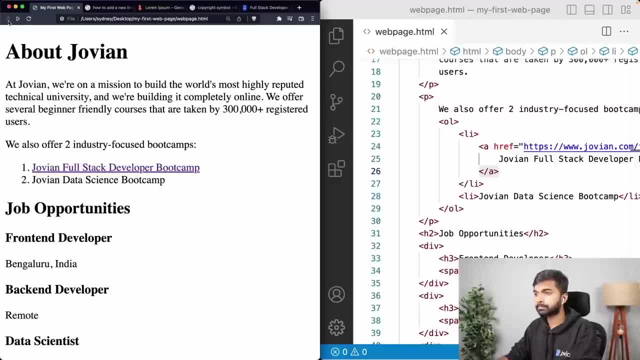 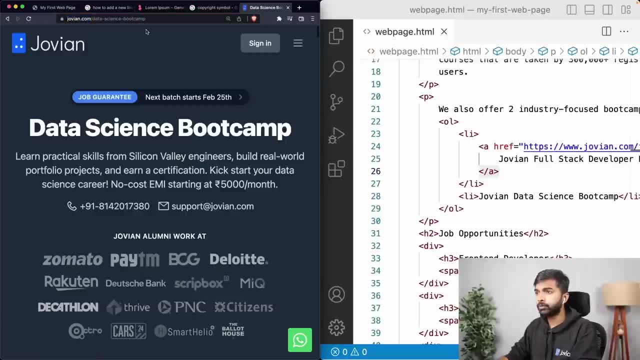 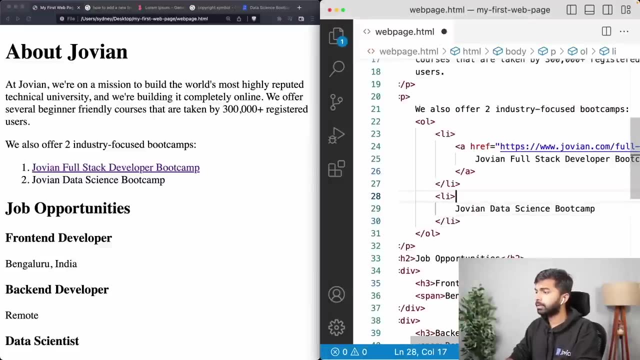 on. this is going to take me to the full stack developer boot camp page. Great, Let me grab the data science boot camp page as well. So data science boot camp: copy that link And once again, let's put that on a new line. Let's create an, a tag here, a. 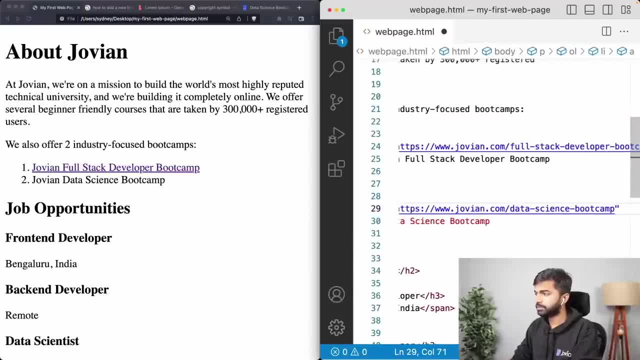 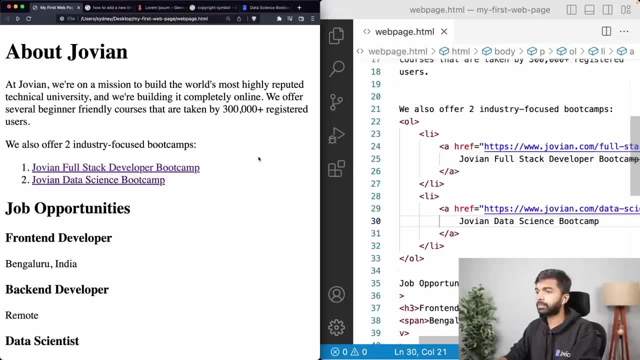 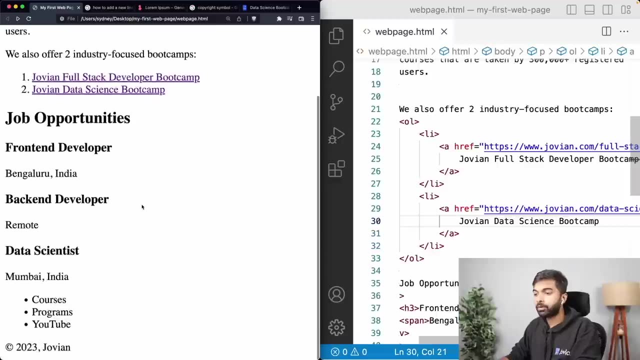 href equals: oops, yep, data science boot camp. And let's take the closing a tag and let's put it here And let's save that. And now we have the Jovian data science boot camp linked from here as well, And that is how easy it is to add links within a web page. Let's go ahead and maybe let's. 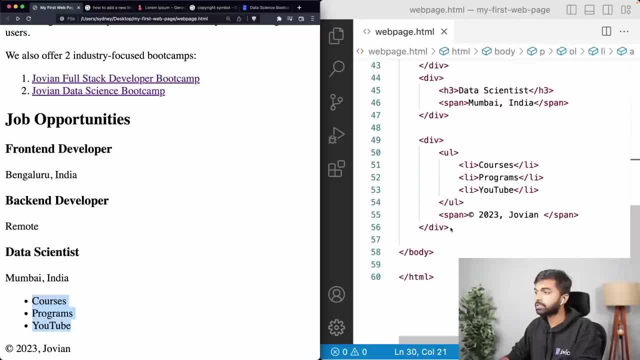 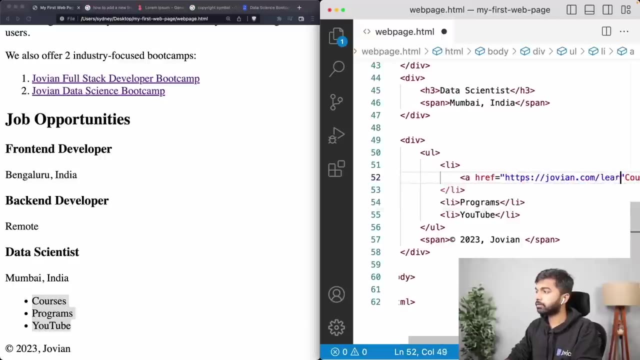 also link a bunch of these footer links. So I'm going to come in here and I'm going to say: let's see a href equals. Let me just point it to joviancom slash learn for now. Yeah, All right. And let me also point the second one to joviancom slash learn. 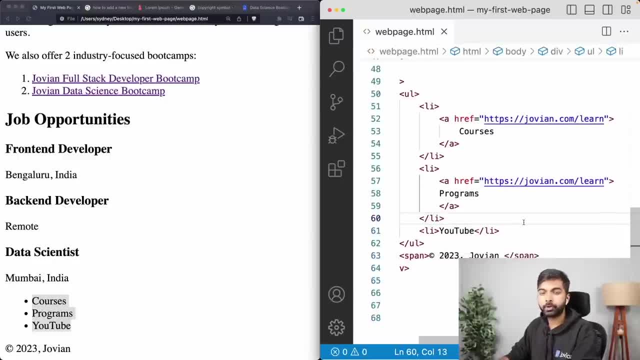 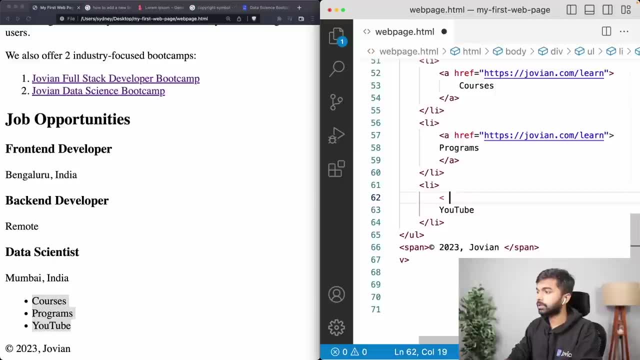 Okay, so both the courses and the program footer links for now are just going to go to the same page: joviancom: slash learn. And then the third footer link- let me point that- to our YouTube channel. So a href equals gdps. youtubecom at Jovian HQ. 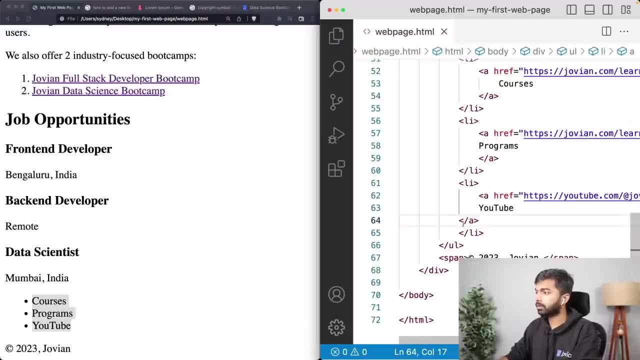 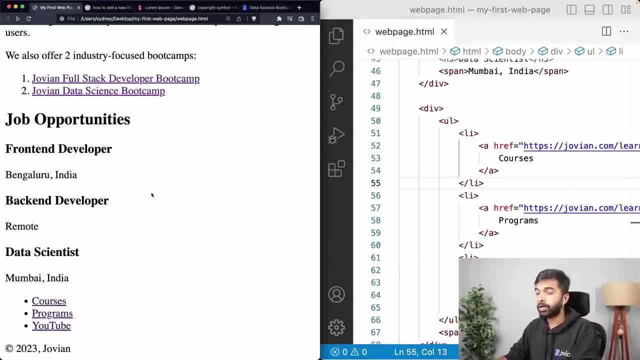 Okay, Let me just format that. So let's say format document, and that's going to just indent things a little better. All right, so now we have this courses link that opens the courses And we have the programs link that opens the programs. 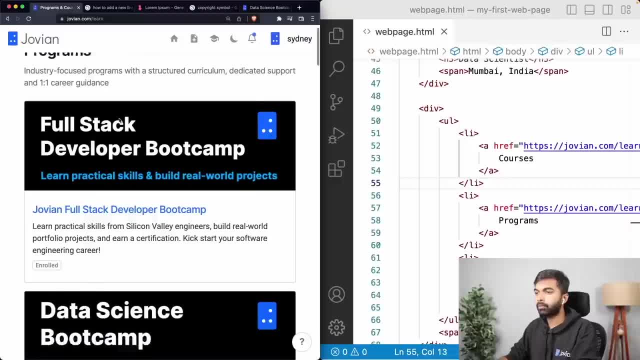 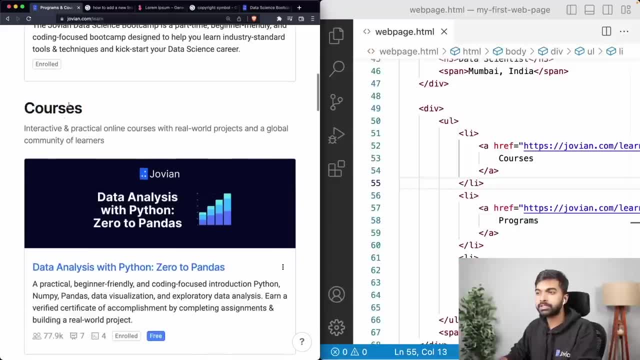 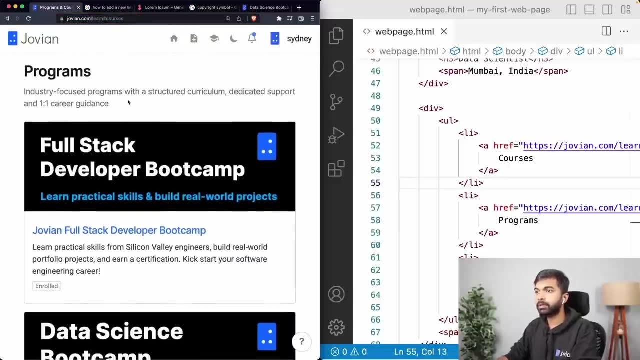 But of course both are going to the same place. But what we have here is this particular section within the page. it actually has an ID. So the section has an ID called courses. So if we actually type something like this, hash courses at the end of the URL. Okay, that doesn't seem to. 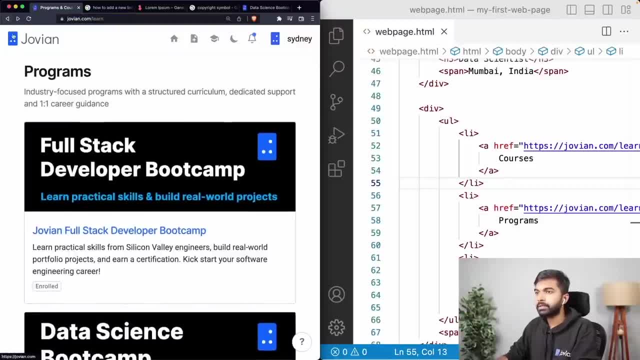 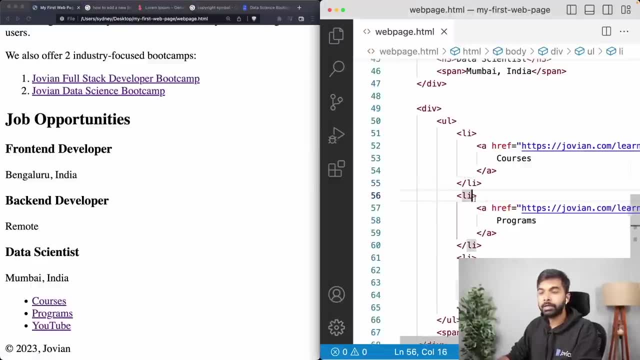 work. Yeah, So yeah, we have linked the courses, we've linked the programs and we've linked the YouTube channel. Now, one thing that I want to do here is I also want to add a new. I want these links to open in a new tab. I don't want to change the current tab. 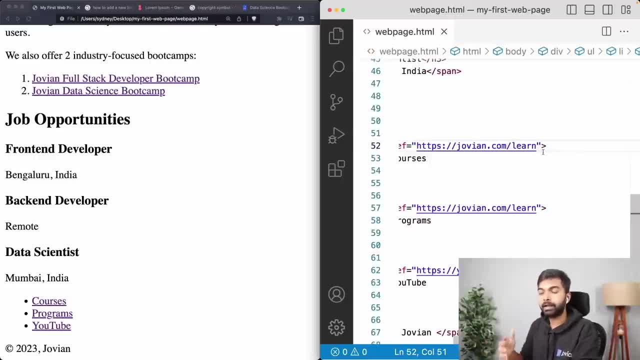 because somebody is looking for jobs. I don't want to get distracted and lose track of the jobs page, So I'm just going to add target equals underscore blank. Okay, So anytime. what does this mean? What is underscore blank mean? Why do you need that? 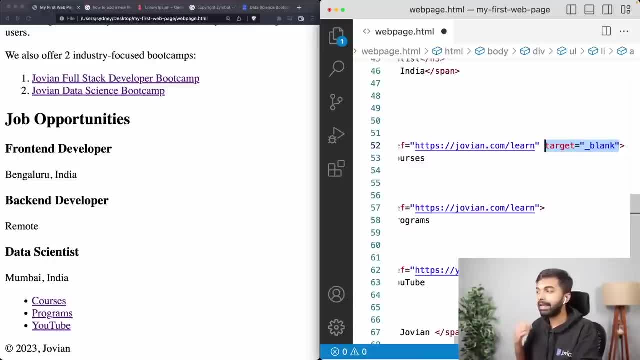 underscore. don't worry about all that. this is a very standard syntax. anytime you need to open a link in a new tab, just put target equals- underscore, blank, as an additional attribute in your a tag. okay, that's all it is used for um. there are other targets that are possible as well, but underscore. 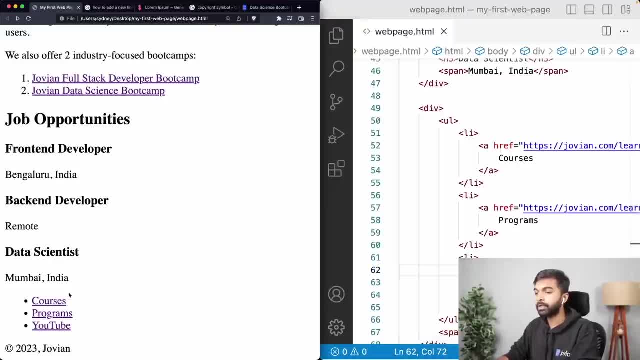 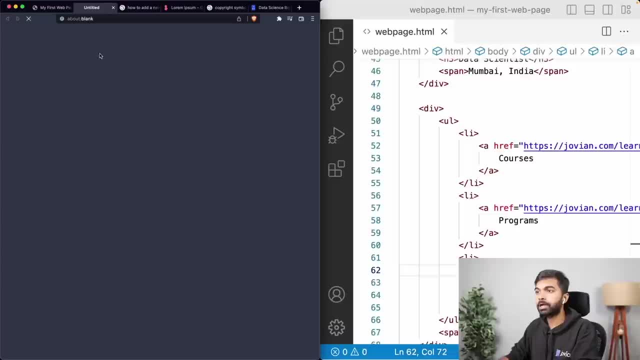 blank is typically what you should be using in most cases. okay, so now if i click on courses, that is going to open it in a new tab. okay, then, if i click on programs, that is going to open it in a new tab. if i click on youtube, that's going to open it in a new tab. all right, so now we've. 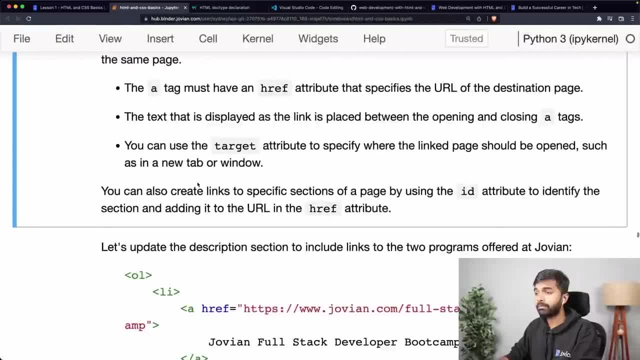 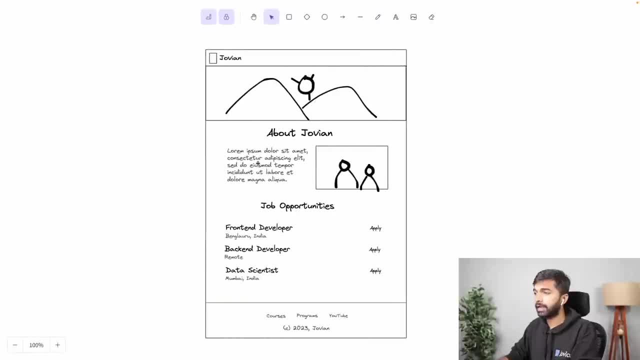 added links and our page is shaping up quite well. now we have links on the page as well. what next? what else is missing from our page? so we've added headings, we've added some text, we've added some um jobs as well. uh, we've added footer links. i think the images are missing. 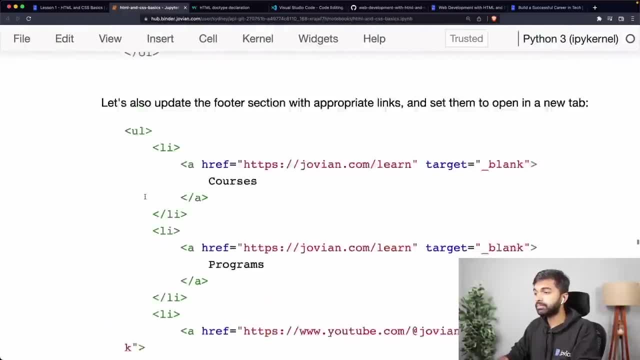 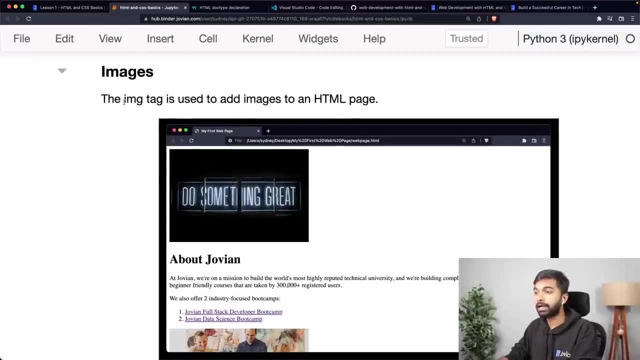 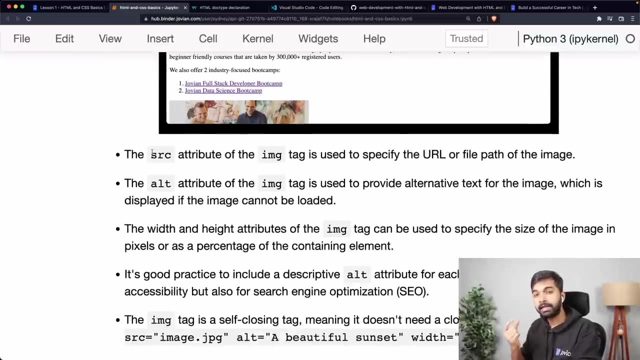 so let's add the images as well. how do you add images in html? well, so the way to add images in html is using the img tag. so there's a tag called img and you can use that to add images. now the- just like links, are added using the a tag. a is short for anchor, so links are. 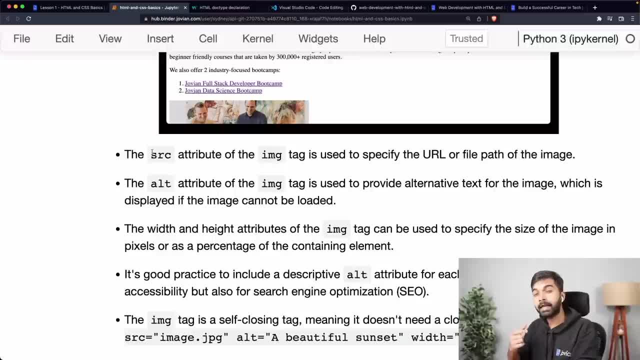 added using the anchor tag or a tag and you have to specify an href attribute. similarly, images are added using the img tag and you can specify the src attribute with the location of the image. the image could be on your computer. the image could be next to the web. 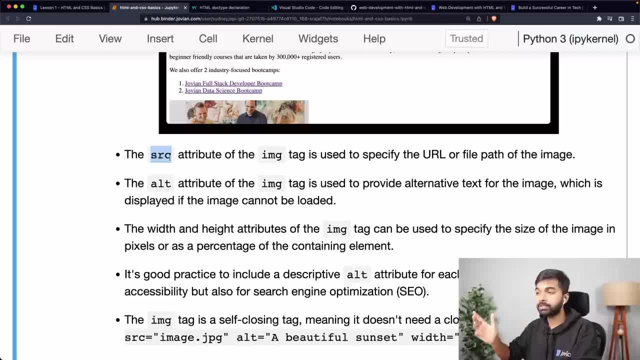 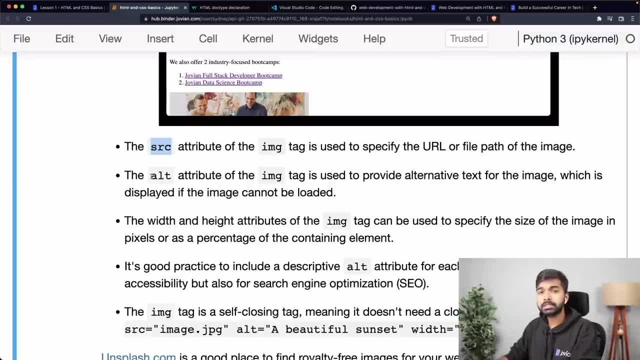 page, basically, or the image could be somewhere on the internet. both of these work. you can just specify the location of the image using the src attribute. apart from that, because images also typically have, you should also indicate what that image is about. this is for screen readers and for search engines, etc. so you can also add an alt attribute or an alt attribute which is: 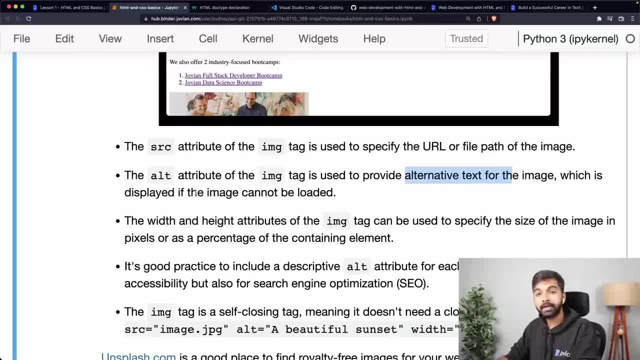 used to provide an alternative text for the image which is displayed if the image is not loaded, and also read by screen readers for people who are unable to see the image, and it is also read automatically by search engines to improve the visibility of your page on search. 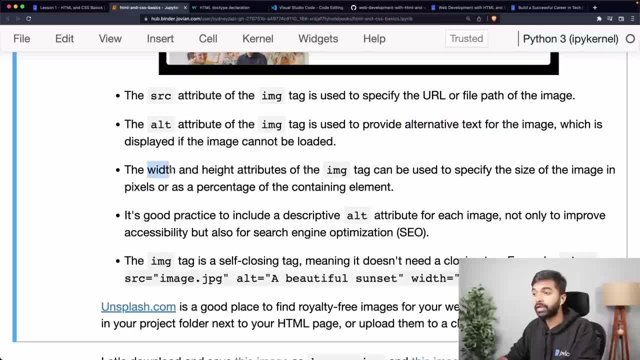 Now the width and height attributes of the image can also be set using the width attribute and the height attribute, and you can specify the width or height of the image as pixels on the screen. So if you know the resolution of your screen, the resolution of your screen is typically- 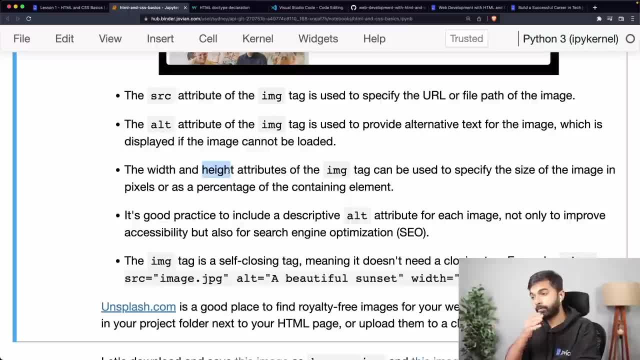 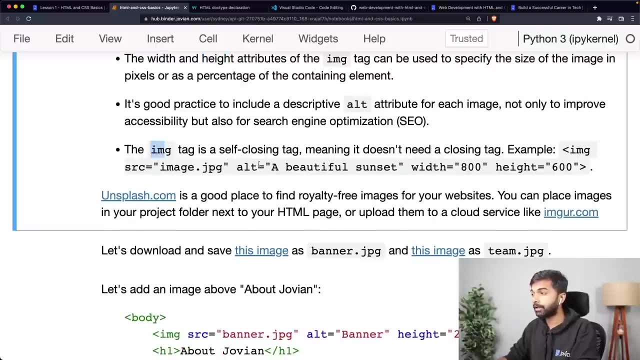 given in pixels, for example, 1280 pixels horizontally and 720 pixels vertically, something like that. So you can specify the height and width of the image in pixels as well. Okay, now the last thing is that the image tag, or the IMG tag, is a self closing tag. 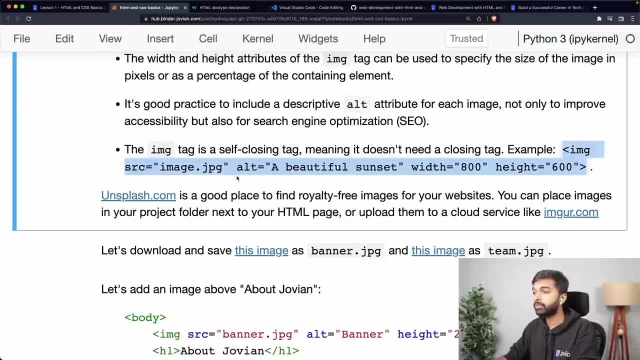 which means that it does not require a closing tag. you just put the IMG tag, you put its SRC, you put its alt attribute, you put its width, you put its height and, if you want, and that's it. You don't have to put a closing tag. you don't have to put anything within the image tag. 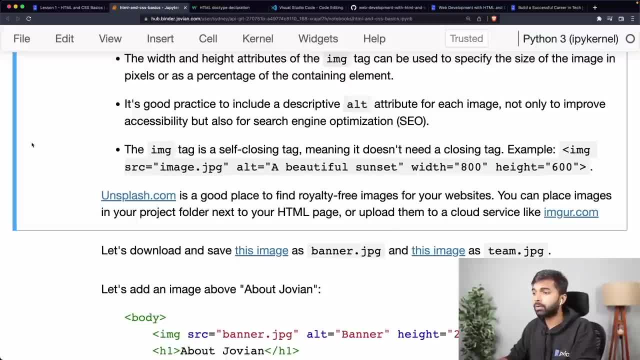 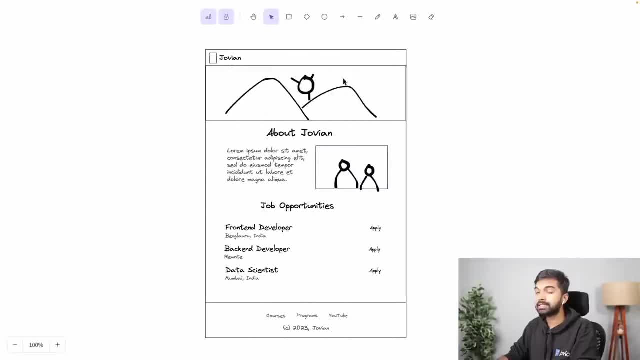 as children. So let's check out some images that we can possibly use. We need a couple of images: one image here as the banner that's going to show up on the entire page, left to right, and one one image here which is going to show up here on the. 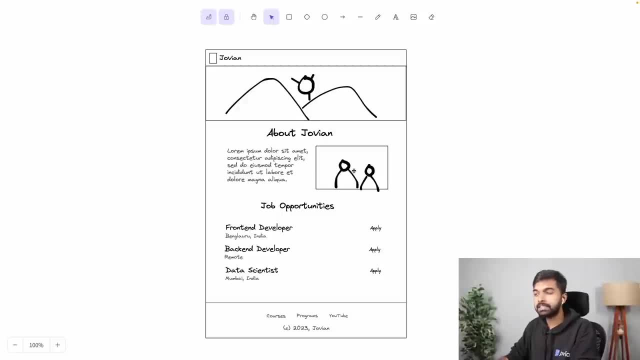 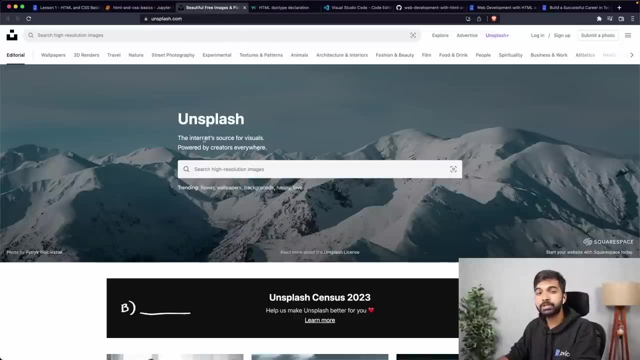 right, Okay, so how can we add? how can you find these images? Well, one good place to find great photos that you can use for free is Unsplash, So Unsplashcom is a great place. I'm going to search for career here. 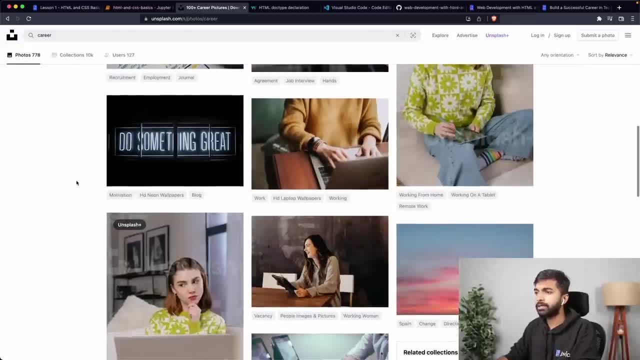 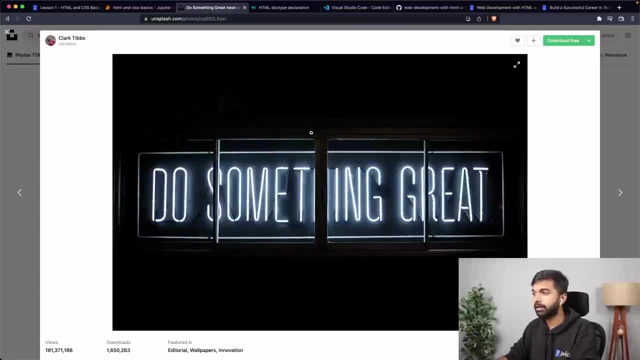 And let me scroll down to find an image that might be good as a banner. I think this image looks good, So this image is a nice image that I could use as a banner on the page. maybe not the entire height of the image, but maybe like just this section would be good. 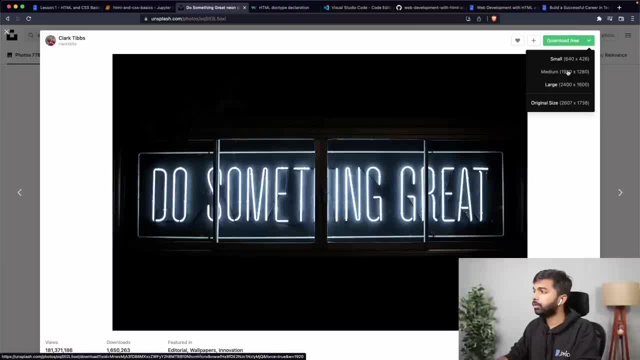 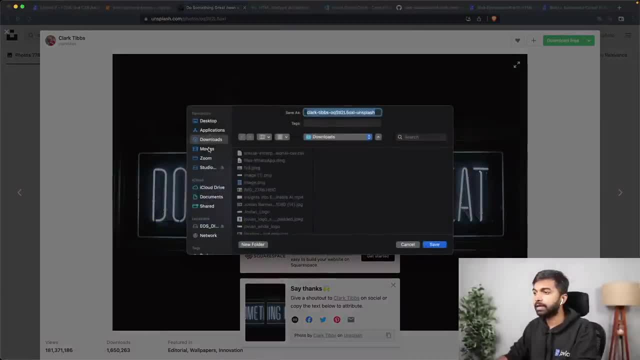 So I'm just going to go here and I'm going to say download free, And from here I'm selecting the medium size. Okay, So that is going to download a JPG file And I'm going to come into my desktop, go into the folder where I actually have the 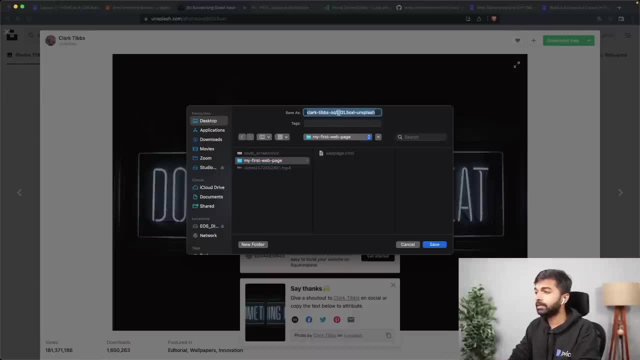 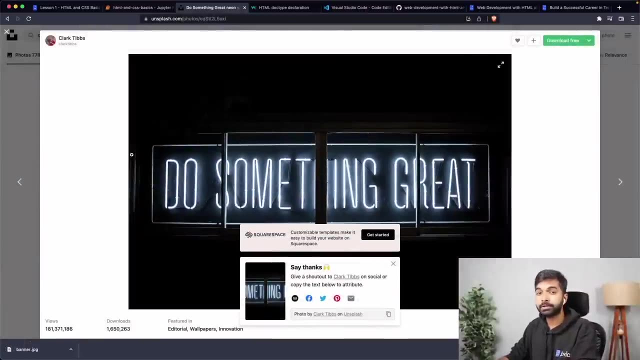 web page or HTML file and put in the image file here, So let me just call it banner dot JPG. Okay, so now we've created a banner dot JPG file, So that is going to be the banner that we use on the page. 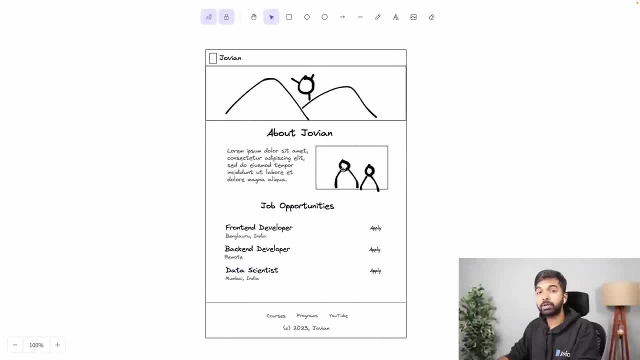 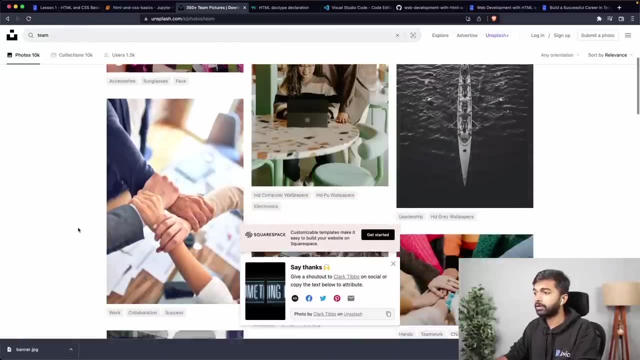 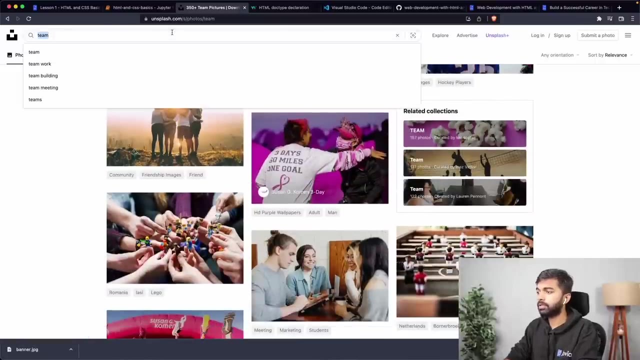 Let me grab another image which is going to show up here, Maybe here I want to show a team picture. So let me close this and let me search for team. Let's see if we can find a good team image. Or let's search for maybe people working. 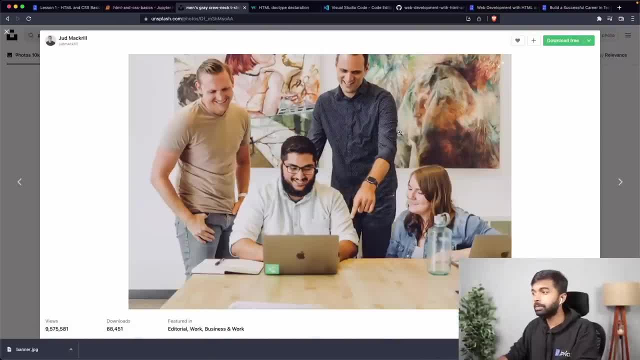 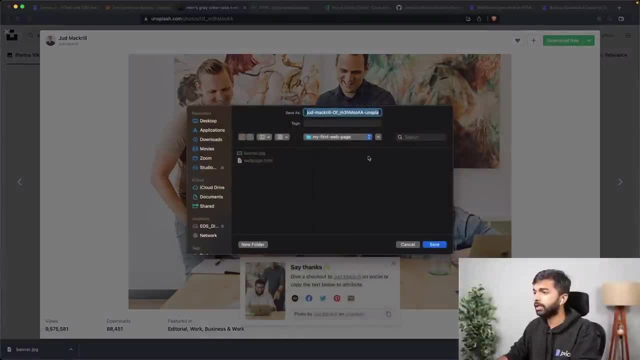 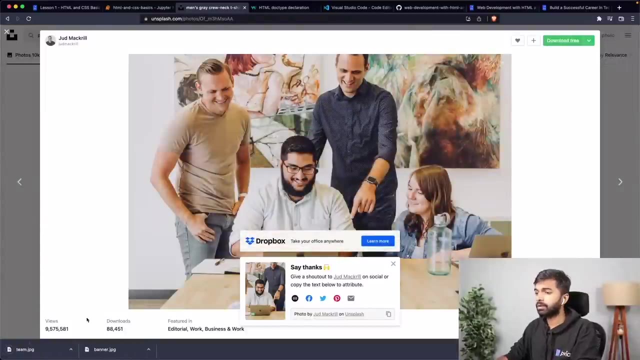 Okay, that looks good. Not the Jovian team, but nevermind, we can still put it on the careers page. So let's download this, also in medium quality. Let's go and call this team dot JPG. Alright, so now, if I open up the sidebar once again, by the way, you can open. 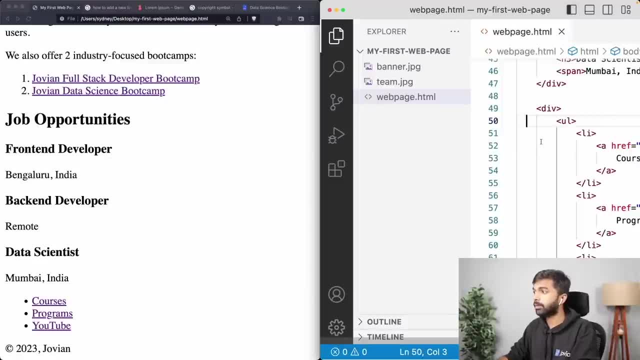 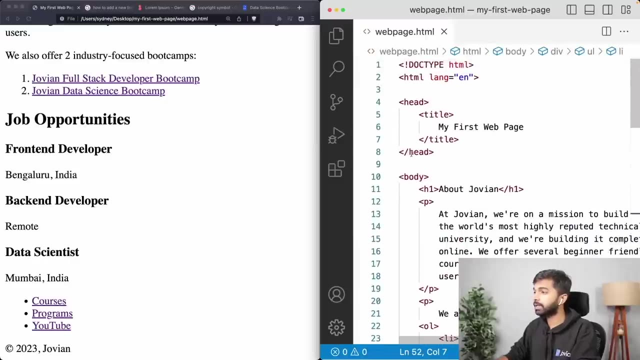 The sidebar, using this button here, or you can also just use command B or I believe it's control B on Windows. you can see that, along with web page or HTML, we now have these files: team dot JPG and banner dot JPG, And now we can add these images into our HTML page. 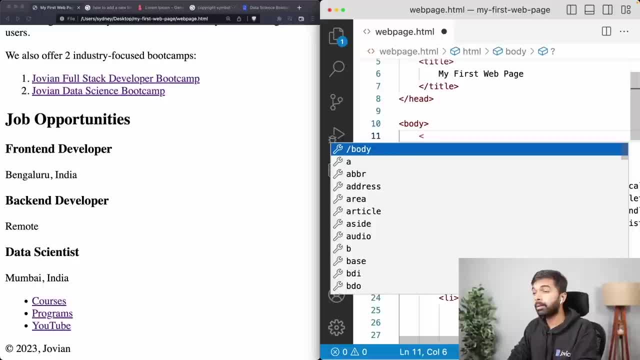 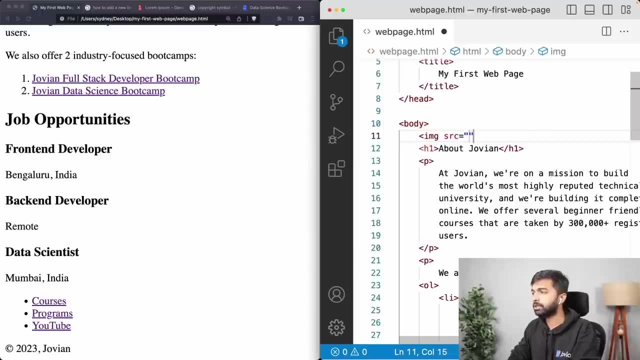 The first image, the banner dot JPG image, is going to show up above the heading about, about Jovian, So I'm just going to add IMG, SRC equals and paste Okay, And I'm going to name the file name here: banner dot JPG. 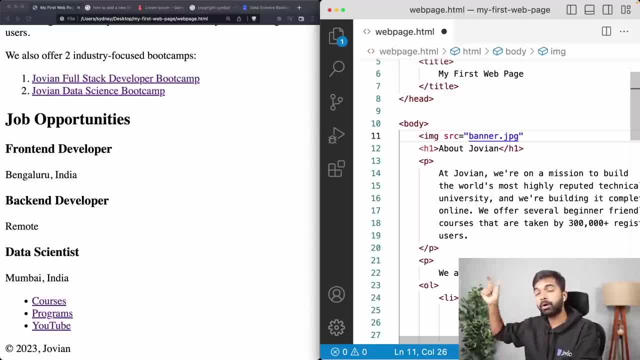 Remember. this could also be a URL of an image on the cloud or somewhere on the internet, But for now the image is right here next to the file that I have, So I can just put that. and let me just put the alt text here. 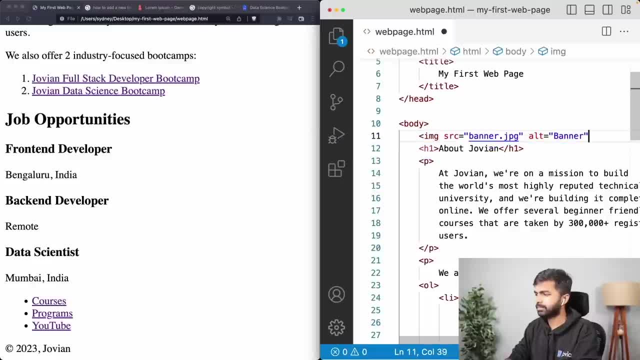 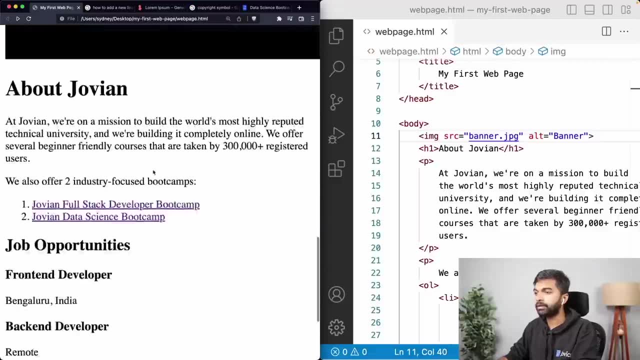 And the alt text I'm going to put here is a banner. this is the banner. I'm going to close this tag. Let me now reload the page and you can see that the image has been added here, but it's too big. 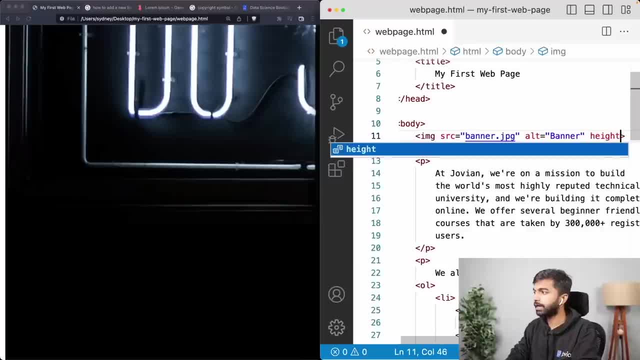 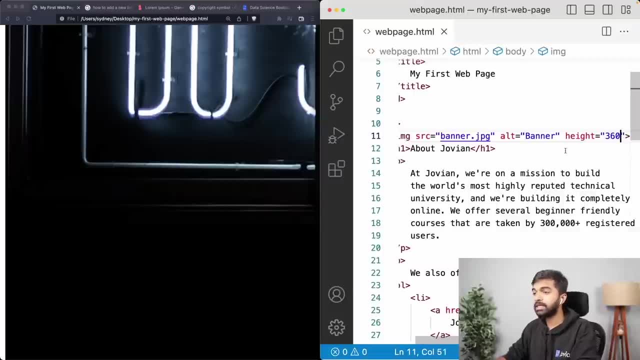 Let me just shorten the image, Okay, Because I'm going to just say height equals and I'm going to set the height of the image to, let's say, 360 pixels. So when I say height equals 360 and reload, now you can see that the height of the image. 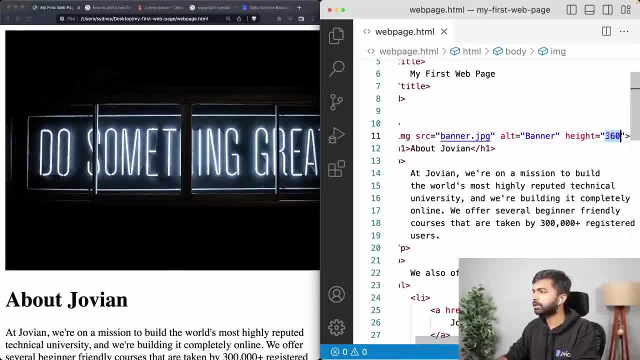 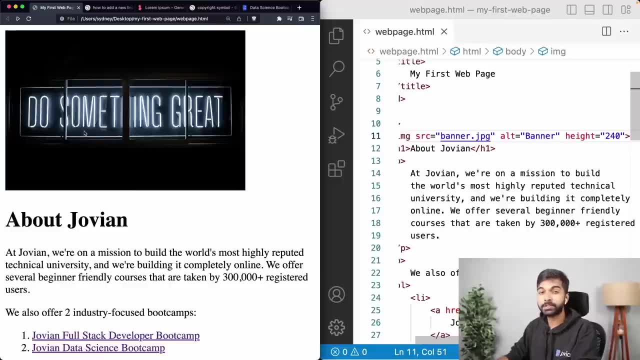 has been reduced to 360 pixels. okay, I can reduce it further, maybe just for now, and we can make it bigger later. Yeah, Now the height of the image has been reduced, So now we have this image. of course, it's not laid out how we want, but it's there in. 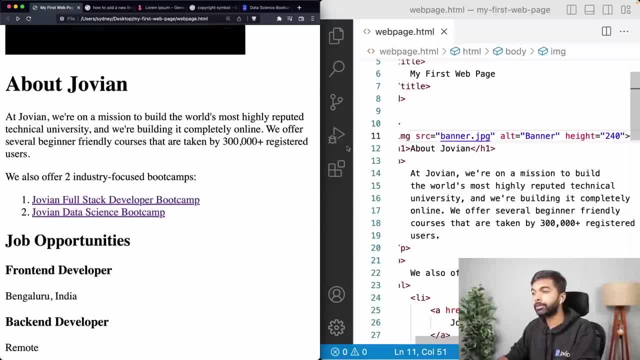 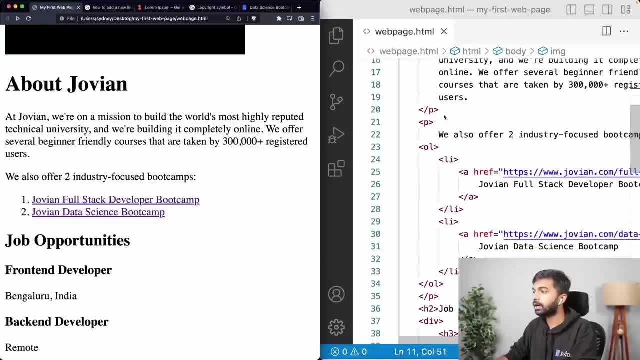 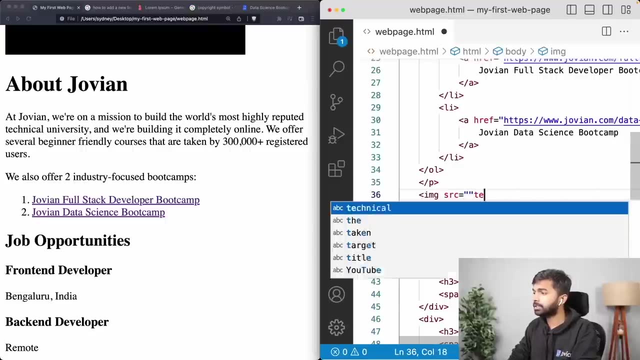 the right place. And then the second team image is going to show up on the right side. So in some sense right is next or after. So I'm just going to put that second image after the speed tag, before job opportunities. I'm going to say: IMG- SRC equals teamjpg and alt equals team. 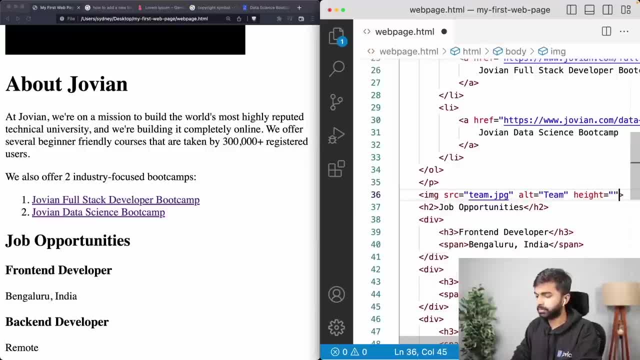 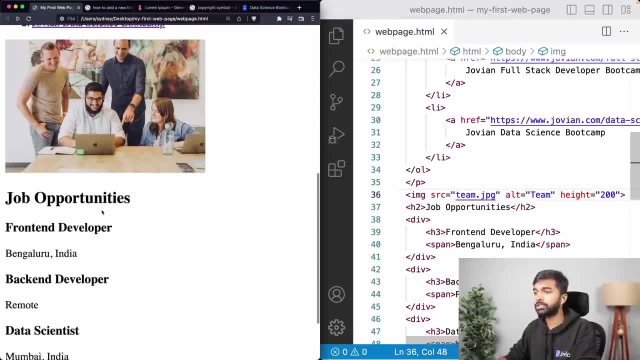 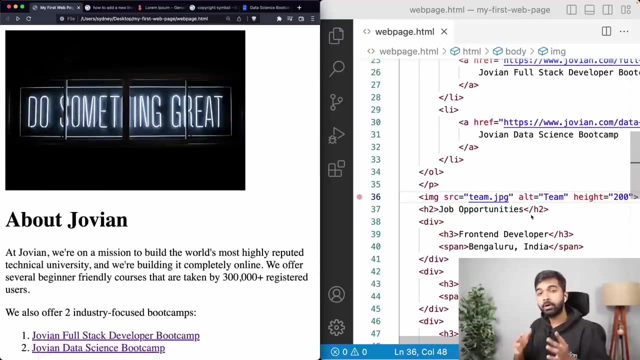 And let me give it a height of 200.. Okay, let's reload that. Okay, And we can see the image here as well. Great, So again you should. what you should be doing is pausing this video, watching maybe five. 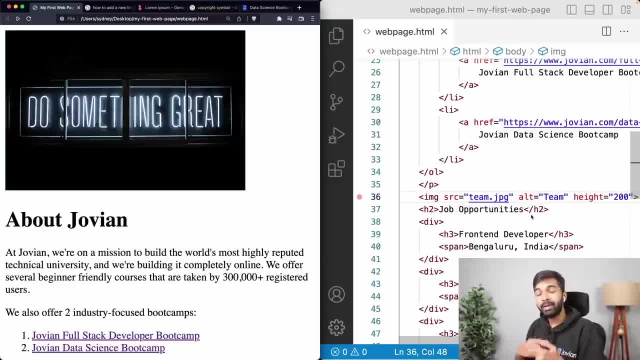 minutes and then following along, typing or everything on your own, and build this step by step. the best way to become a better programmer is to just hold, write a lot of code, And even if you're writing the code that you're seeing on the screen, you should be asking. 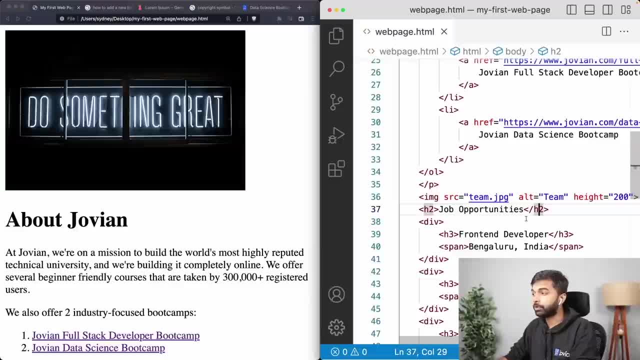 yourself what that code means, And you should be experimenting with it a little bit, And if something breaks, you should be searching online and maybe asking us a question. Okay, that is how you're supposed to do this. It's not enough to just watch this. 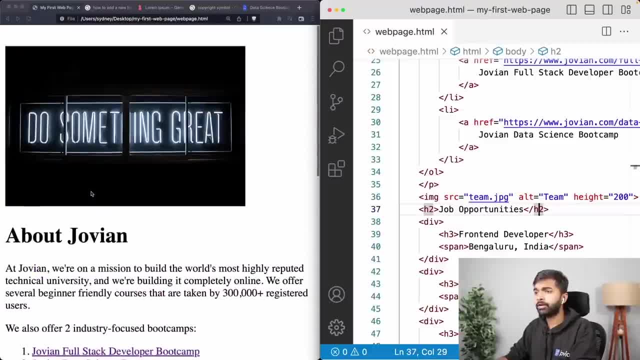 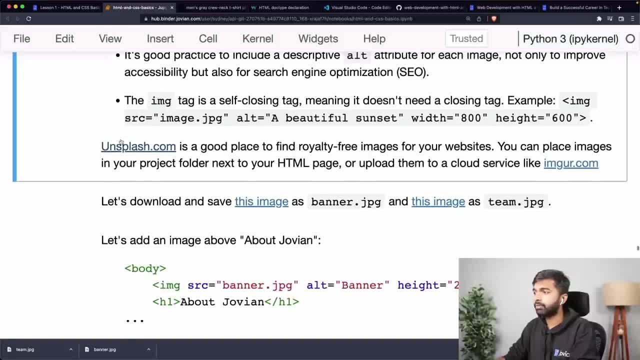 But at this point I feel like we have all the content that we require on the page. It's just not laid out properly. All right, So we have all the content. Let's see. Yeah, we have all the content we needed. 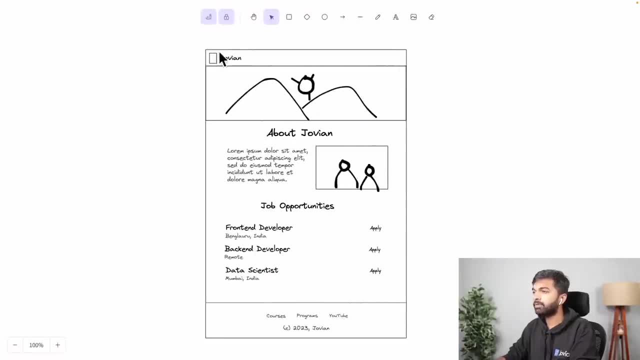 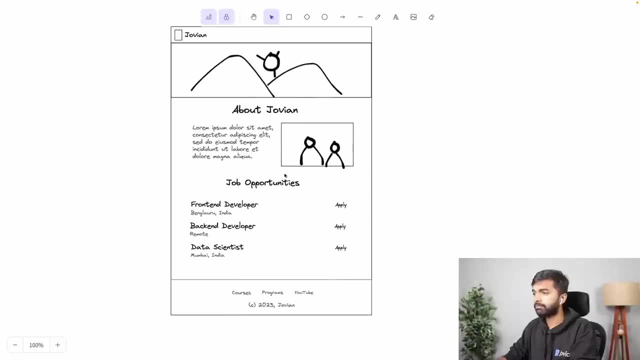 We have this about Jovian. we have this image. okay, maybe we don't have this navbar logo right now. How about we fix that? sometime later we'll we'll figure it out, But we have job opportunities. We have this image here. 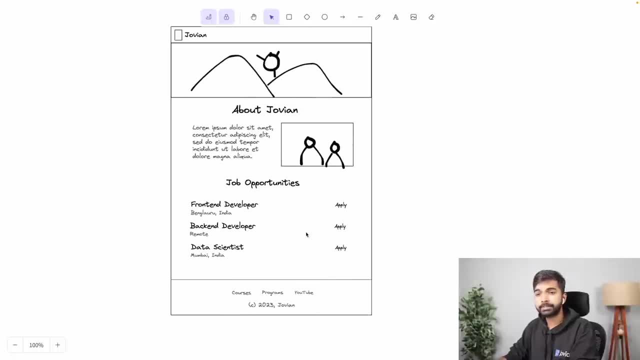 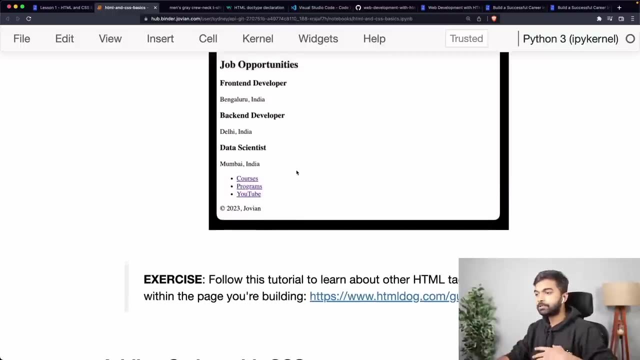 We have this footer, Okay, And we have this copyright section. Now, one thing I want to mention about HTML tags and CSS- HTML and CSS in general- is that there is so much here, so many different tags and everything that you shouldn't go about. 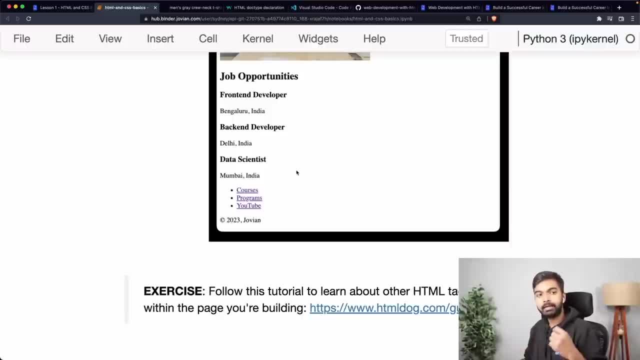 trying to learn every single tag and every single attribute of every tag before you start building web pages, because then you will just be doing that for years. It's you should take the opposite approach, where you start trying to build something And whenever you feel that, okay, you're not able to build it with the tags, you already 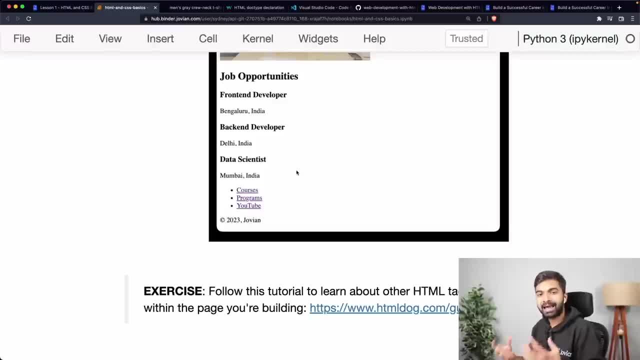 know You can search online to see if there is a certain tag or maybe a certain other CSS property that is going to help you do it, And over time, the things that are going to be used most frequently are going to become second nature to you. 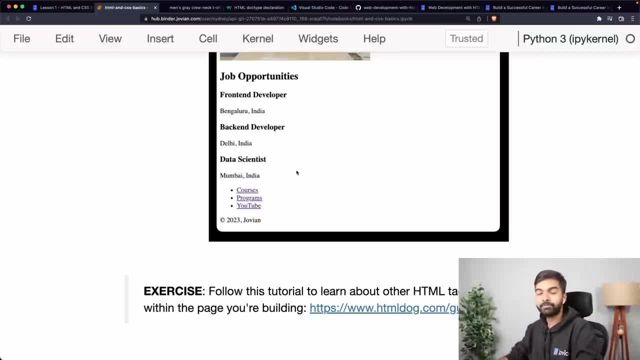 And you won't need to look them up. That is what I do. I still look up some fairly basic stuff on CSS, even after 15 plus years of web development, and I do this every week. So one exercise for you is to check out this tutorial on HTML data. 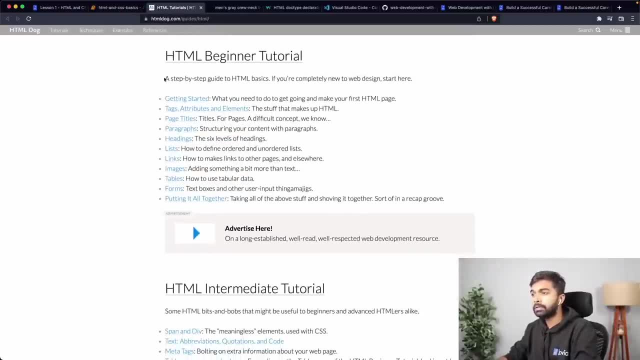 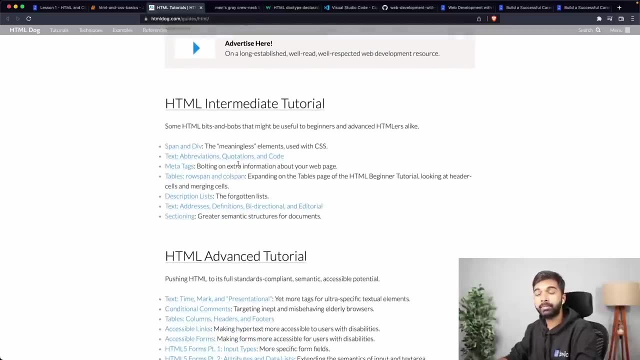 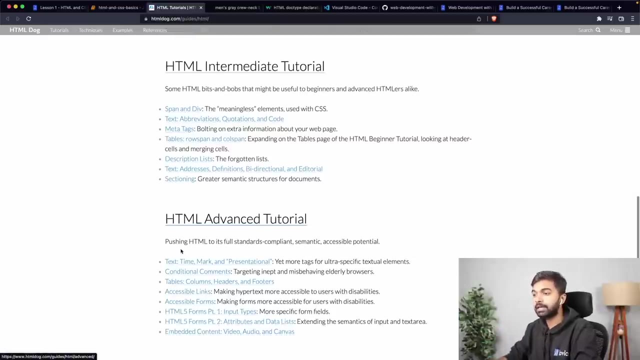 Okay, It's dogcom on the various beginner and intermediate level tags. So you can check out the HTML beginner tutorial in the HTML intermediate tutorial. So once you're done with this lesson itself like this out, at the very least go through all these different types of tags. 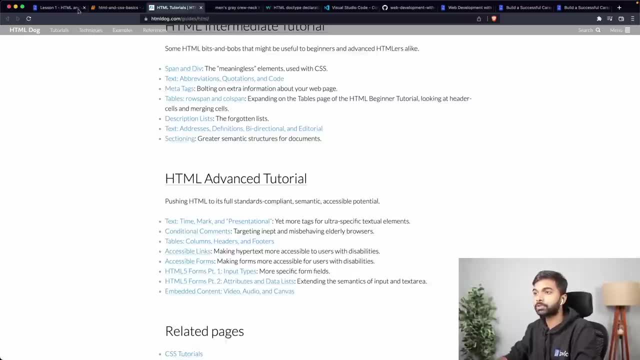 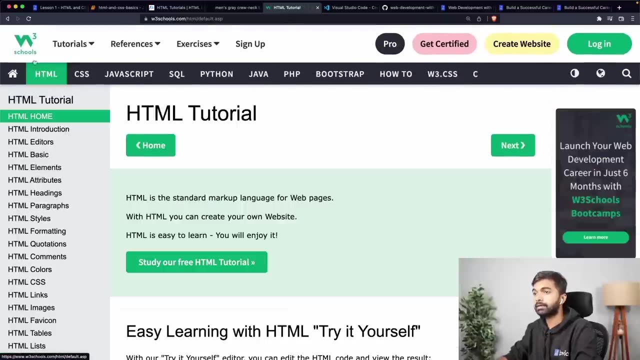 And, if you have the time, you can also go through advanced, but that is something that we're going to cover in a future lesson anyway, But this is a good place for you to practice. another good place for you to practice is the w3schoolscom website. 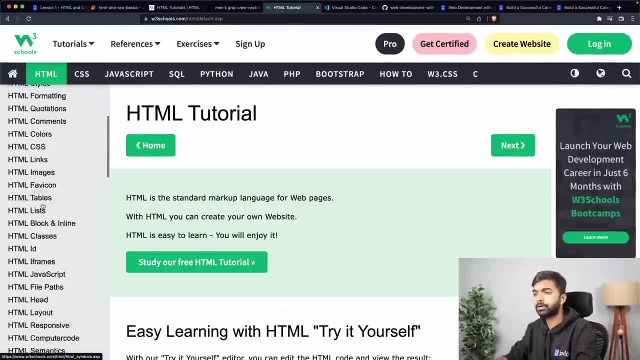 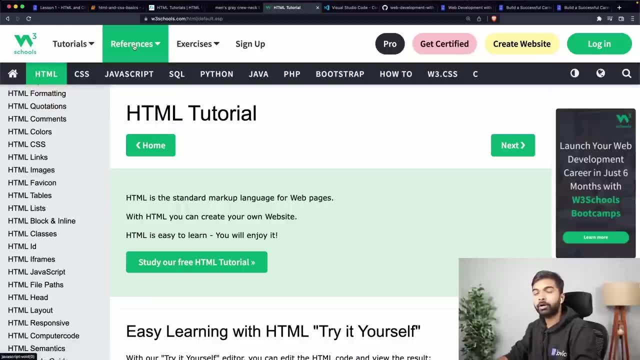 Okay Okay. This contains a great HTML tutorial. So if you want to learn about a specific type of HTML tag, just go find it in the sidebar here and go ahead and do it. We're not going to look at every single HTML tag here, because that's that is defeating. 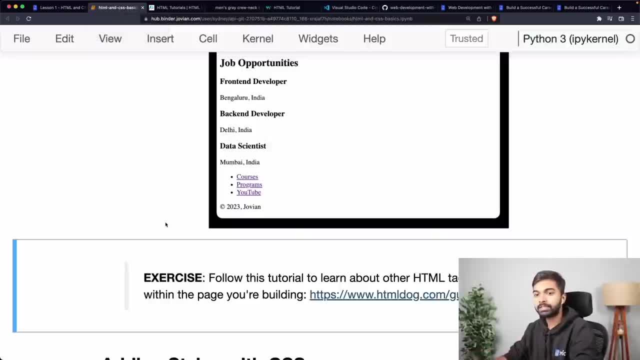 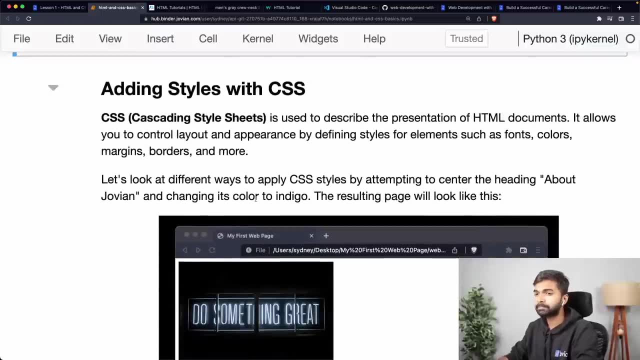 the point. The reason we're here is because we want to build code web pages. Okay, So let's move forward. We are halfway there. Let's go ahead and style the web page Now. cascading style sheets, or CSS, is used to describe the presentation of HTML documents. 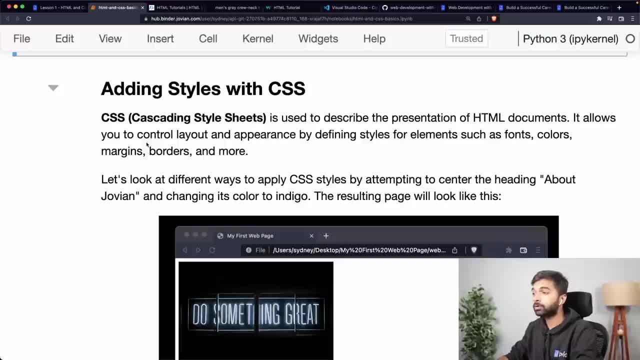 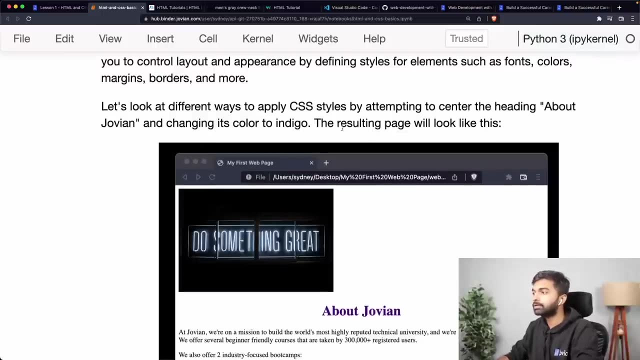 It allows you to control layout and it allows you to control the appearance by defining styles for elements such as fonts, colors, margins, borders and more. So let's look at some different ways to apply CSS styles. There are a few ways to do this by, and we'll do this by attempting to just center this. 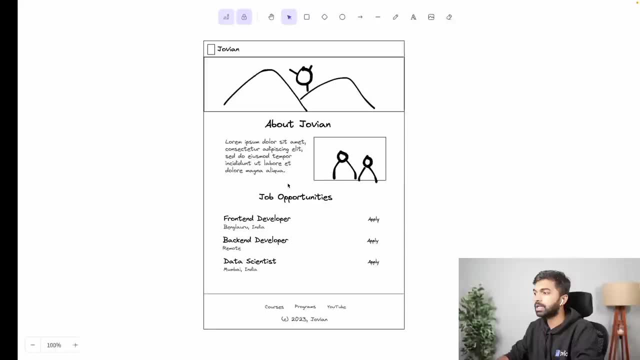 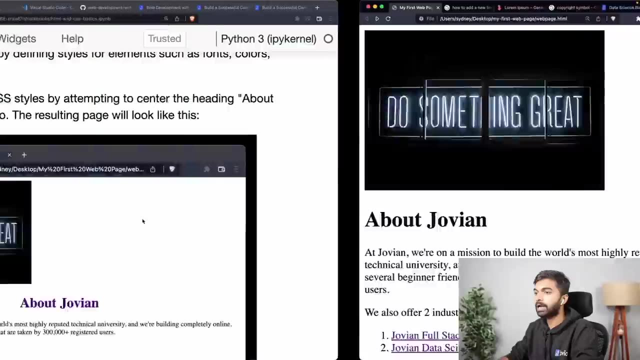 about Jovian heading. we just want to bring it into the center of the page horizontally speaking. we want to bring it in the horizontal center like that, And let's see how we can achieve that Using CSS. So the first way to do it is using something called inline styles. 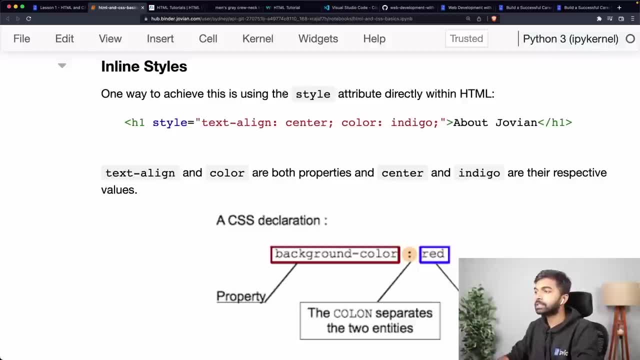 Now, in inline styles, you can achieve this simply using the style attribute And you can put that directly within whatever HTML tag you're trying to style. So let's say we have h1 and we want to style it, So you want to set the style. 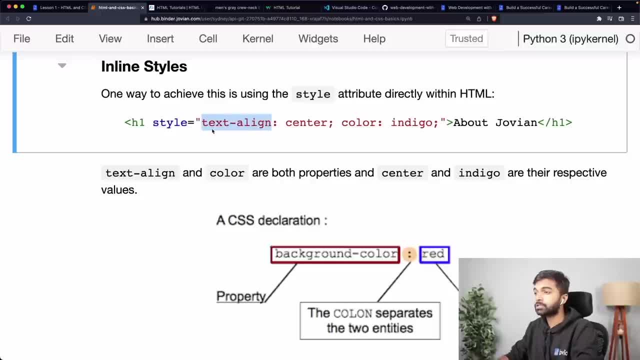 And then, within the style attribute, we want to set this as the value. So this is what a CSS declaration looks like. So what do you do? is you declare certain properties about that tag using CSS. you have a CSS property. So here the property that you are fixing is called text align. 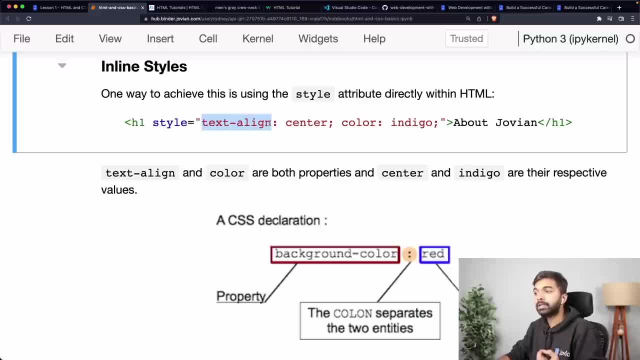 And there are hundreds of such properties. But text align is the property that is used to decide the alignment of the text. should the text be aligned on the left, center or right? And then you have a colon. the colon separates the property from the value, and then you 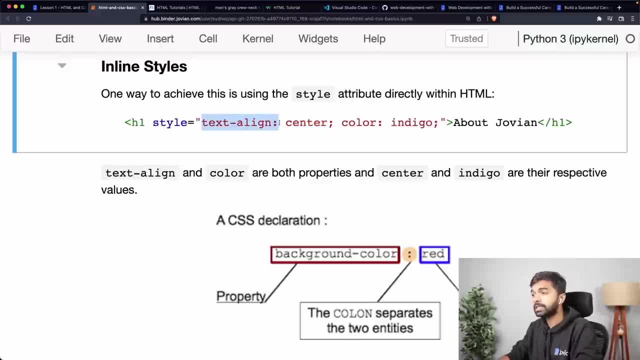 have a value. okay, all of that goes inside the double quotes that are used to enclose the value of the attribute. So yeah, so you have the CSS property and then you have a colon, and then you have the value, And then you have a semicolon to end the declaration. 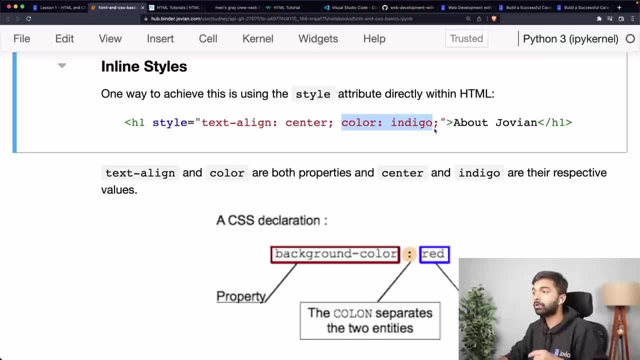 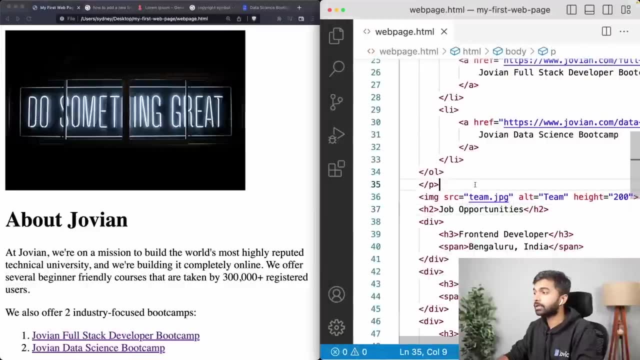 And then you can have multiple declarations here. let's say, apart from centerlining it, you also want to change the color to indigo. that is something that you can do here as well. Okay, so that is the simplest way to apply each apply CSS to some HTML tags. you simply 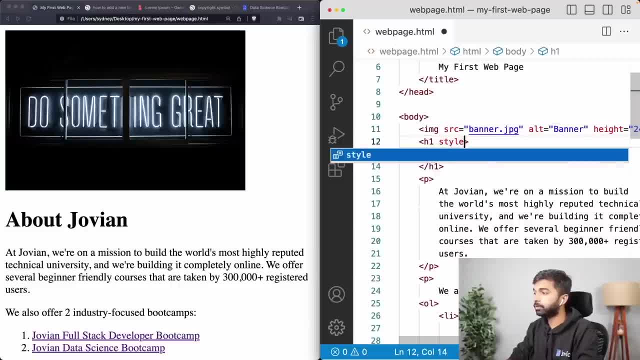 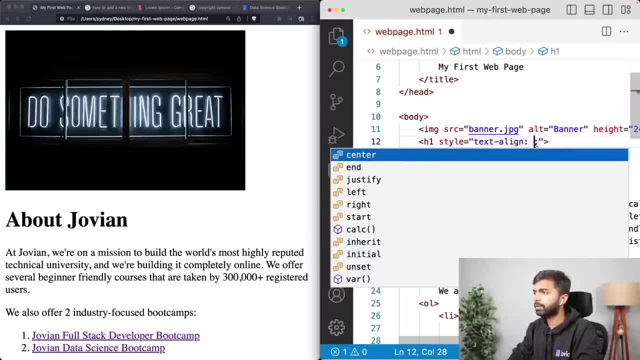 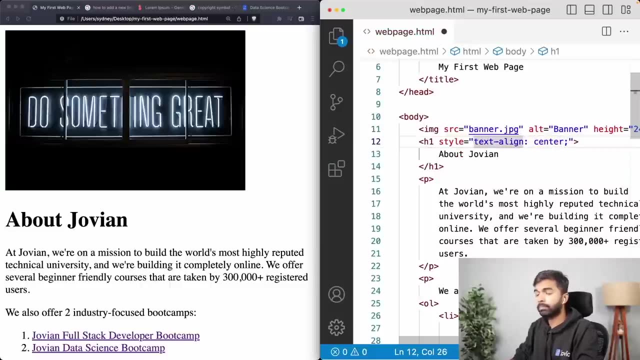 go into the HTML and then you add a style attribute. Now, within the style attribute you add a property. So let's say we want to do text align And for now let me put center here, And then you put: so you have the property colon, you have the value generally, CSS values. 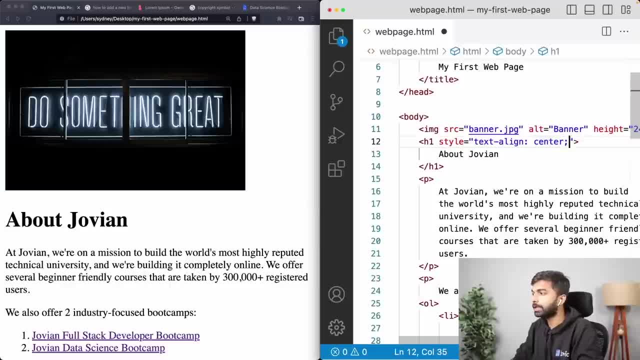 do not require code quotations. some of them do, most of them don't. And then you put a semicolon and let me save that And let's just reload that here And just like that this is centered. you can experiment, you can go and change this. 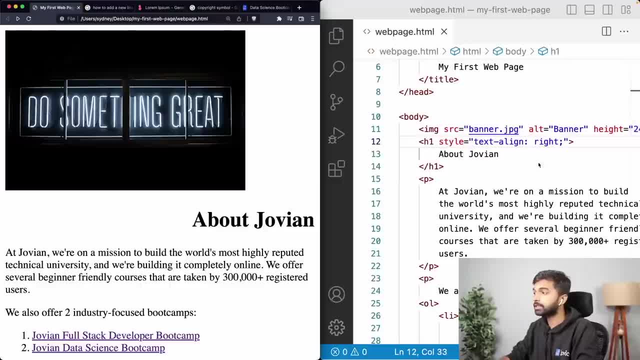 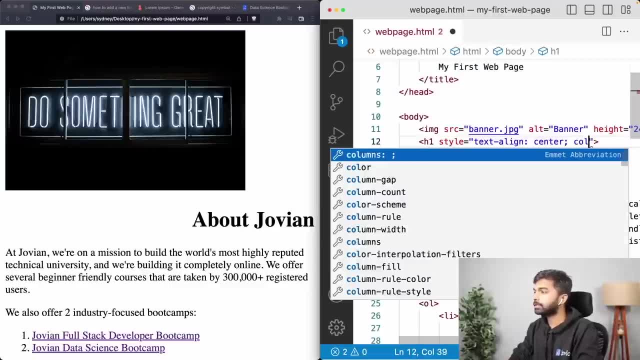 to right And you can see that that should bring you to bring it to the right of the page And again you can go back and change it to center and that should bring it to the center of the page. Okay, let me also add a color. 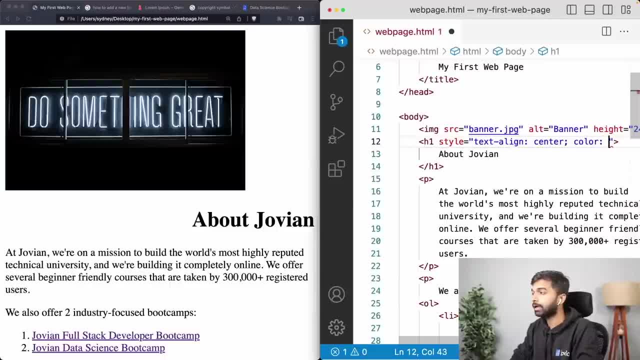 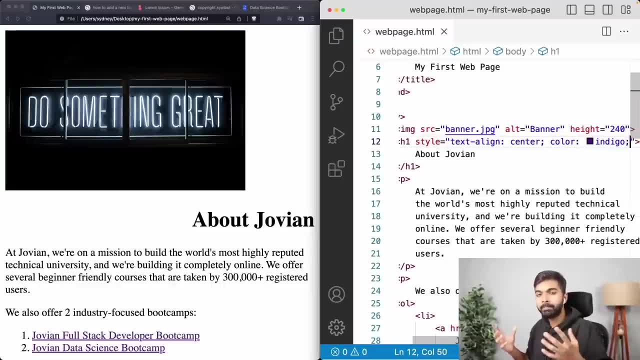 So color is added using the color attribute, And let me set the color to indigo. you can create any color you want using something called an RGB or a hex formula, But there are some named colors within CSS And you can always look these up. 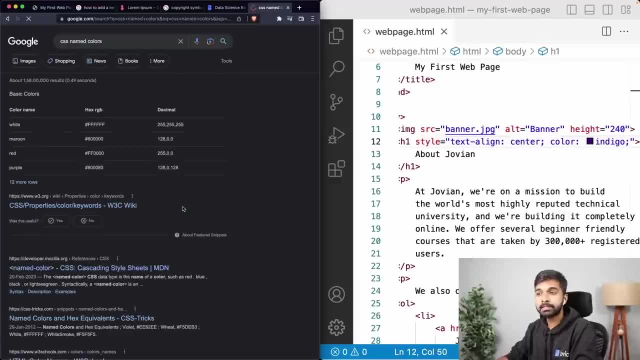 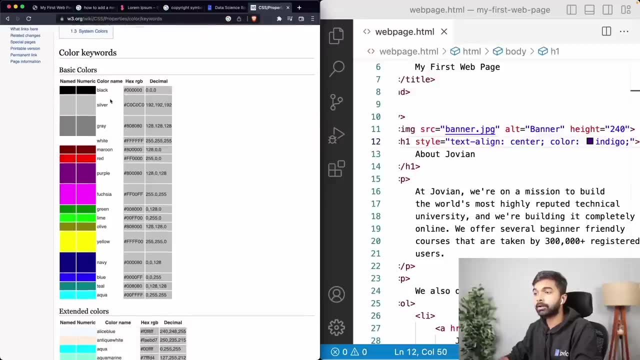 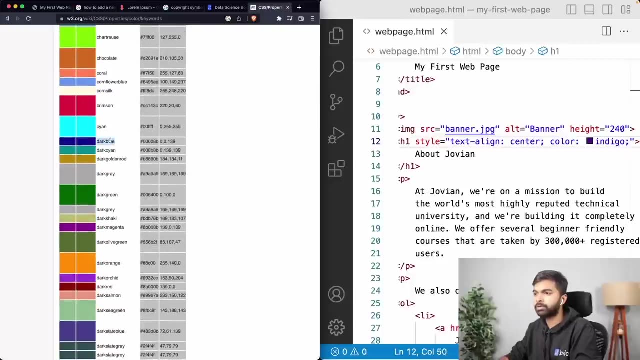 So you can search CSS named colors. So these colors are recognized by every. These colors are already recognized, recognized by every browser. So these are all the colors that are already available in CSS And you can use all of these color names whenever you want, directly. okay, for example, I could. 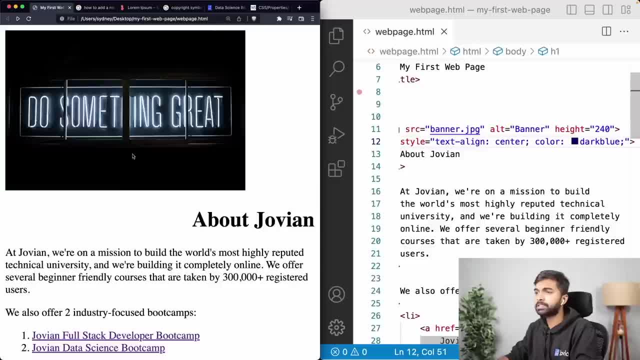 use dark blue instead of indigo, And that would work as well. And let me just reload the page here. You can see that now the content is centered on the page. just the about Jovian heading is centered on the page and it has the color dark blue. 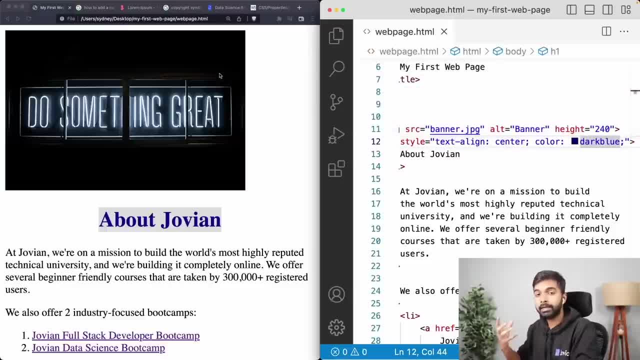 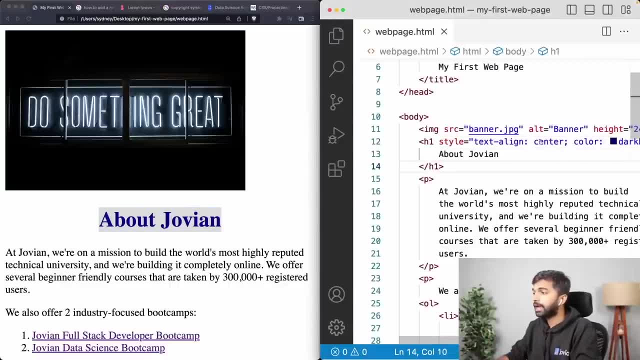 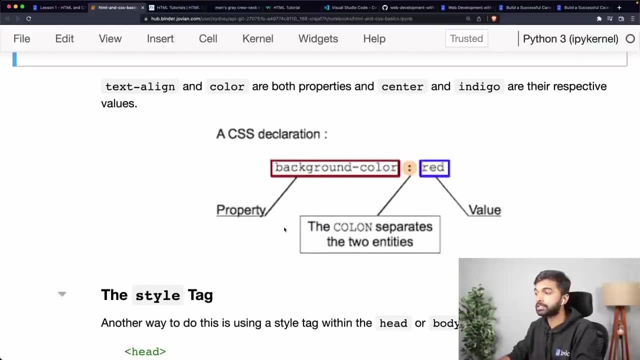 If you want to create colors that are not named already in CSS, then we'll talk about that in the next lesson, All right, All right, So that is one way to add styles. This is called the inline style, And you simply add a bunch of CSS declarations in the style attribute. 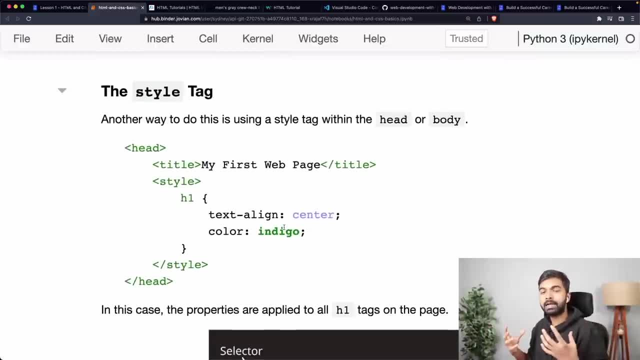 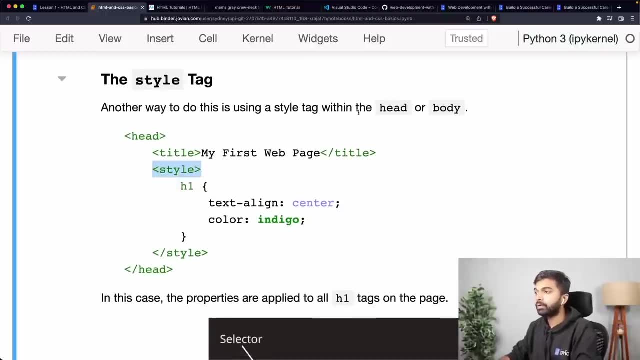 The other thing- because you might want to add a bunch of different styles or you might want to add the same set of styles to multiple tags- is to use a style tag, So you can create a style tag within the head or the body And then you can put some CSS code within the style tag. 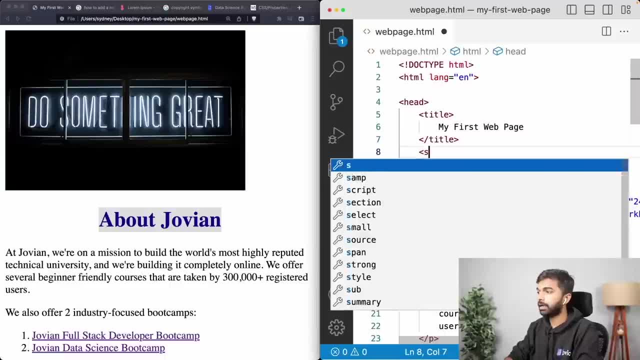 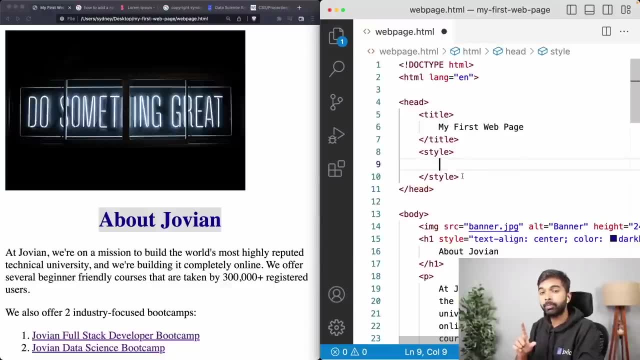 Let me put the. let me create a style tag within the head here. So I'm just going to create style. And now, inside the style tag, the first thing you need to put in is a selector, because now you no longer know where you want to apply the style to and like this attribute, which 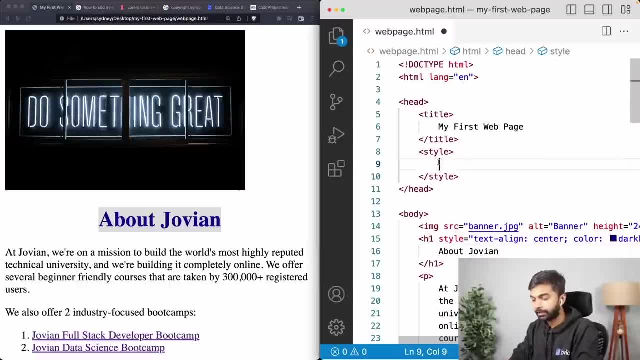 was associated with a tag already, So you need to put in a selector. okay, So there are many ways to select a particular or a bunch of HTML tags on the page. the easiest way to select a bunch of tags: Okay, So you can do this by the tag name. 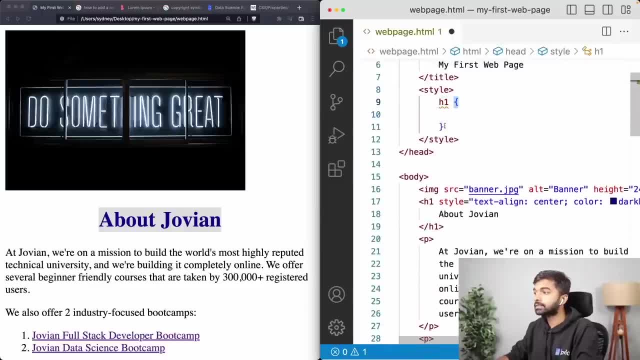 So when you say h1, and then you open these braces or curly brackets, what you're saying- that whatever I put within these curly brackets or these braces should be applied to all the h1 tags on the page. Now, of course, here we have just one h1 tag. 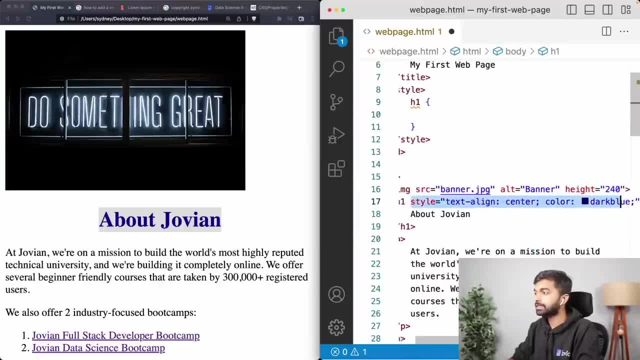 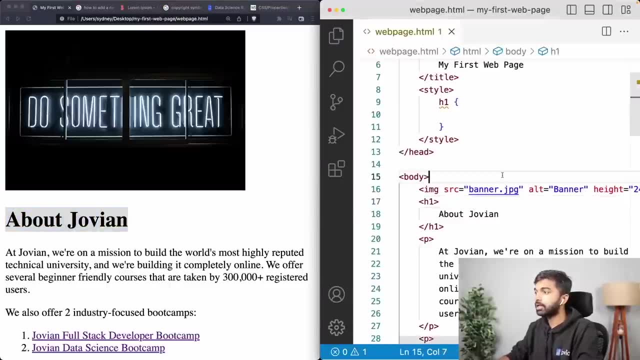 But if you had multiple of those then it would apply to multiple h1 tags. But let me get rid of the inline style here. So now that the inline style is gone, you can see it's back to this position And now in the style tag. 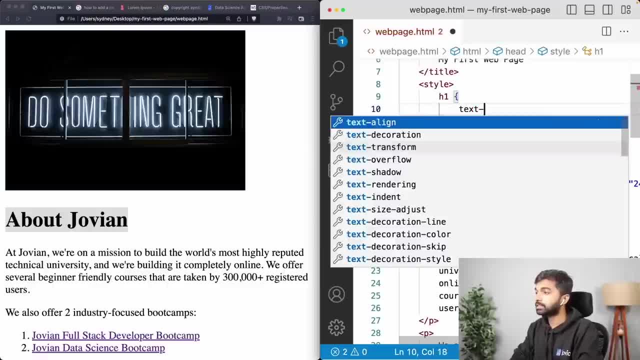 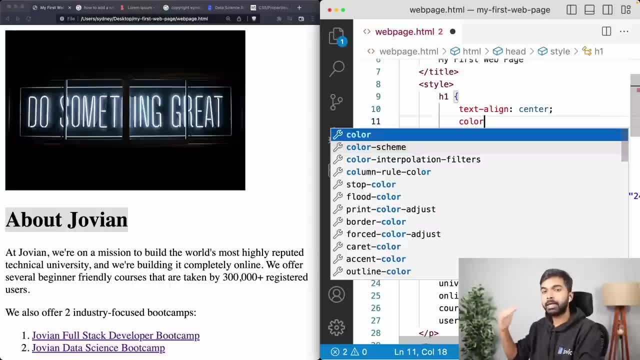 I'm just going to write text align center. And now. one of the benefits of using a style tag is you can use multiple lines. you can make your code easier to read instead of stuffing a bunch of styles within the same attribute and color. 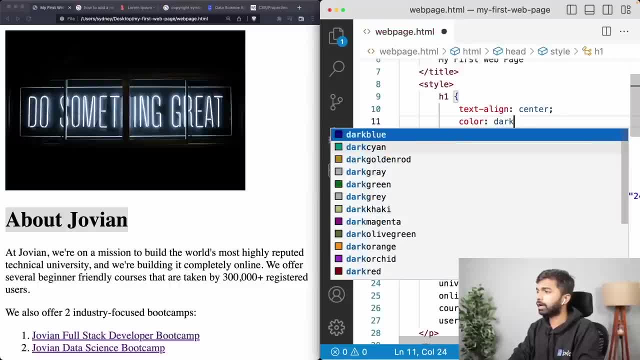 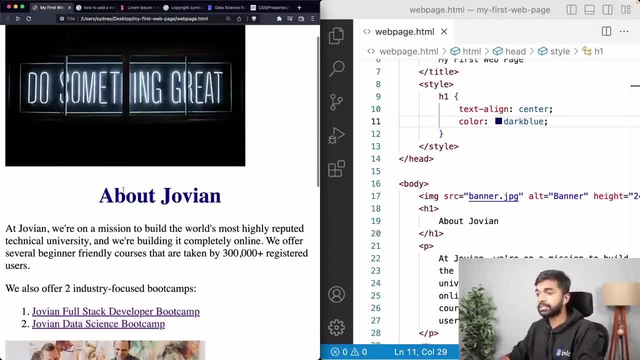 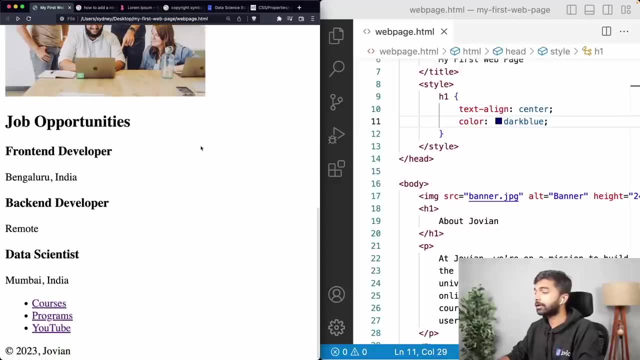 What was that? deep blue or dark blue, Yeah, Okay. so now we have about Jovian, which is at the center of the page horizontally, Okay, And it has the dark blue color. Now, notice that this style did not get applied to any other element on the page. 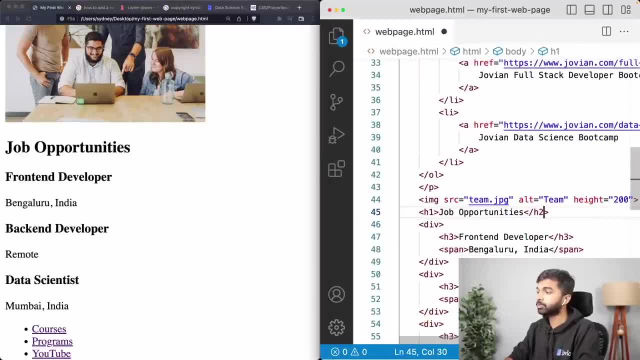 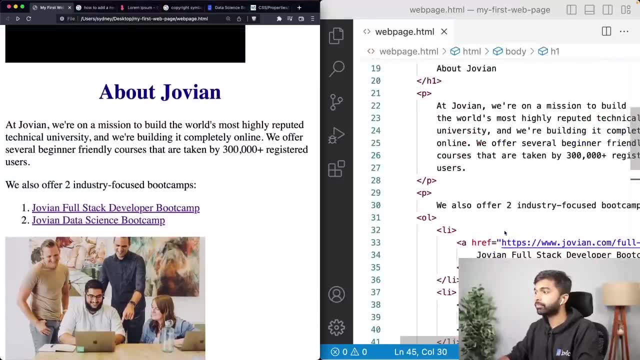 But suppose this second element on the page, job opportunities, was also an h1 tag? you will notice now that job opportunities is also receiving the same style that the first h1 received. Okay, so that is the benefit of using the style tag. you don't have to retype the same. 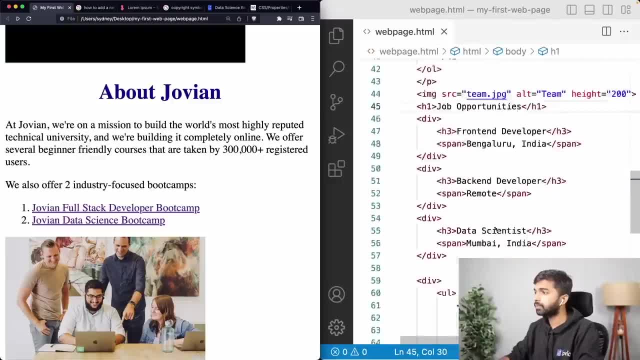 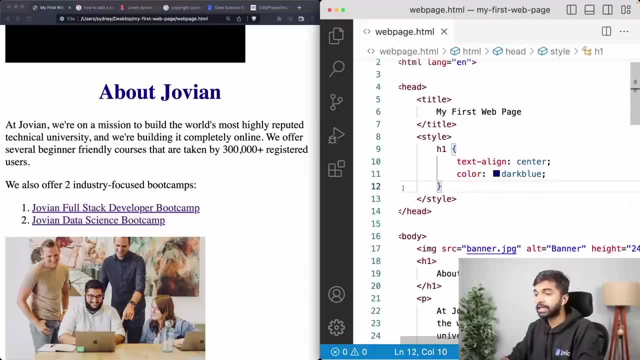 style over and over for each tag. But let's revert that back for now. We are going to make this an h2. Okay, so that is the second way to do it, which is: let's just revert that. Yeah, this is fine. 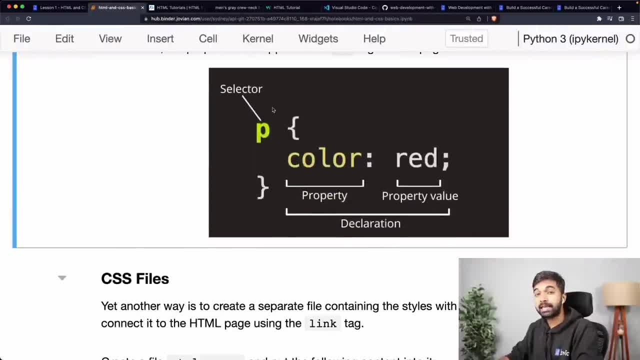 That is the second way to do it, which is using the style tag. So in the style tag you have a selector, And then you have this bracket, and then you have a property, and then you have a property value- Okay- And then you close the bracket. 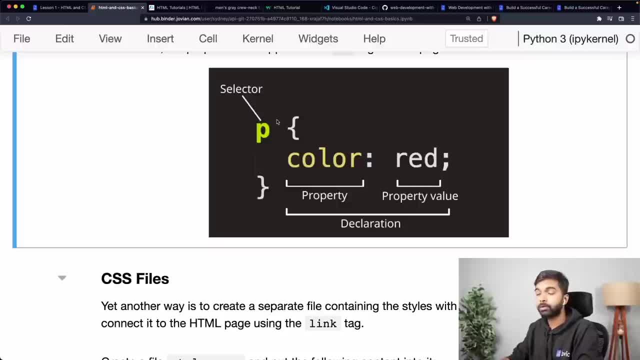 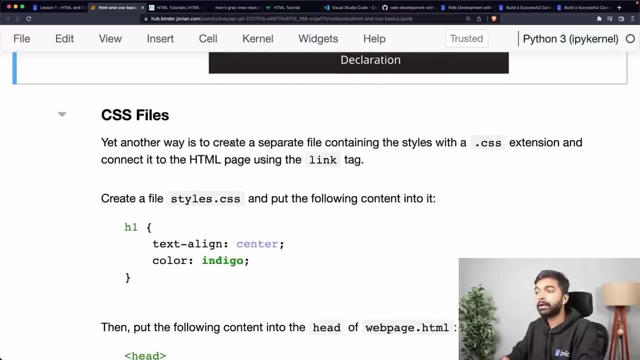 And, of course, you can have multiple properties that you can apply using to the tags that have been selected using the selector, and the simplest selector is just a tag. we look at other selectors as well. Now, yet another way to create, to apply CSS to an HTML file is to create a separate file. 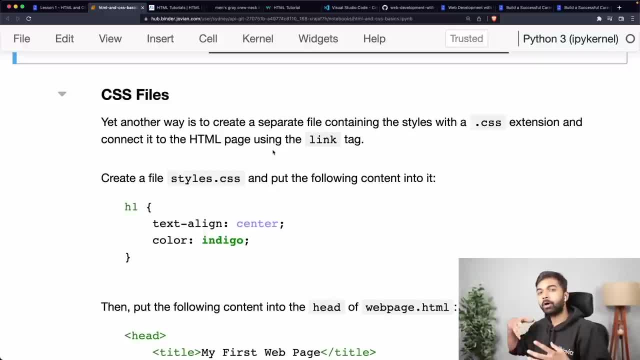 containing CSS. This is very popular because that way you can put all your styles in a single file and all your HTML in a single file And then link the file. link the dot CSS file within the HTML page using the link tag. okay. 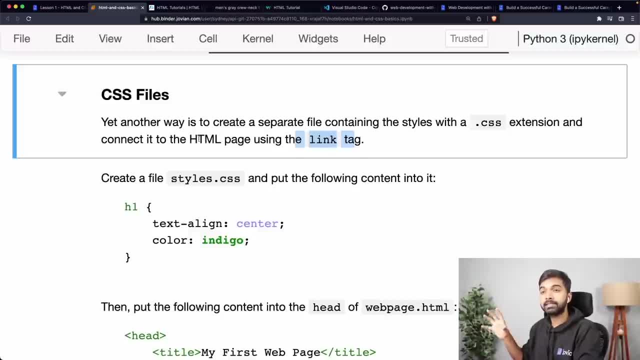 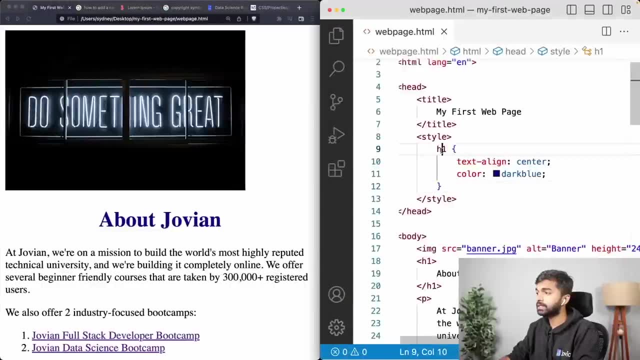 so you use a link tag to specify within the HTML page that the styles should be picked up from this particular CSS file. So let's do this. Let's create a file: styles dot CSS. Let's first get rid of this h1, all of that. 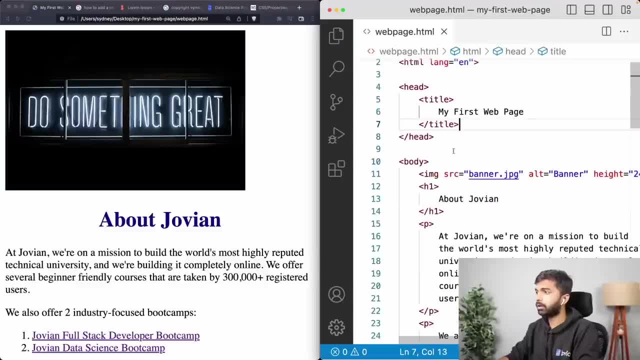 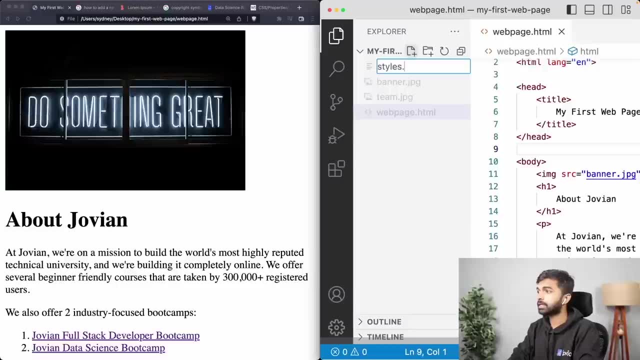 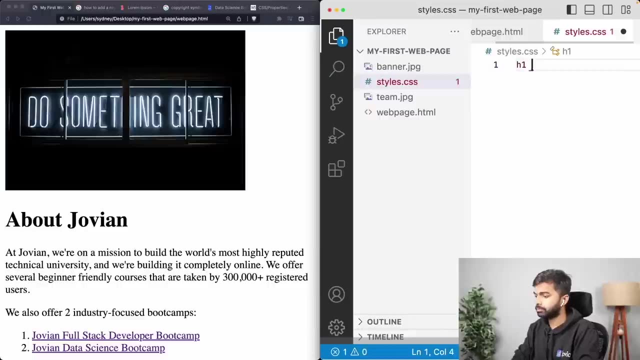 And let's get rid of the style tag. Okay, And you can see that the style is gone. Now let us open up the sidebar once again and let us create a new file, files dot CSS. And now, in this styles dot CSS file, let us add h1.. 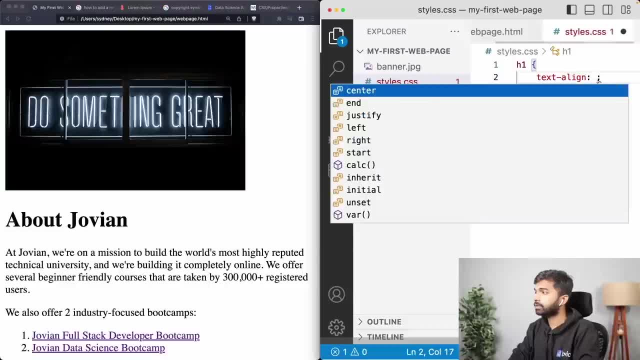 And let us put text align Enter: Okay, Okay, And let us put color: Dark blue: Okay, let's save that And let's reload the page. Nothing happened because we've not connected the CSS file with the HTML file. 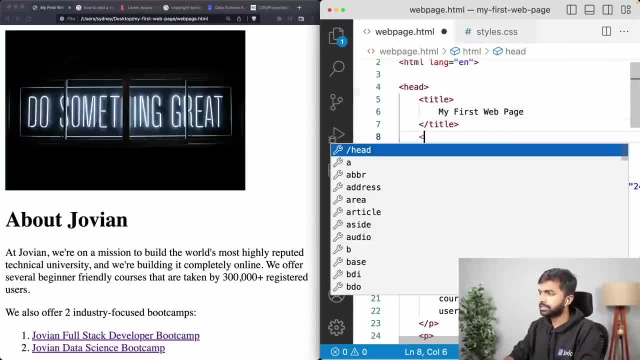 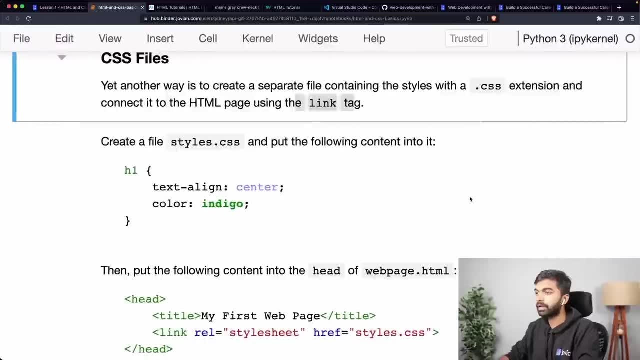 So let's come back here, And now I don't need the sidebar anymore, Let's add a link here. So link is a tag. special tag is typically used for adding style sheets And it has a structure like this: So you say rel equals style sheet. 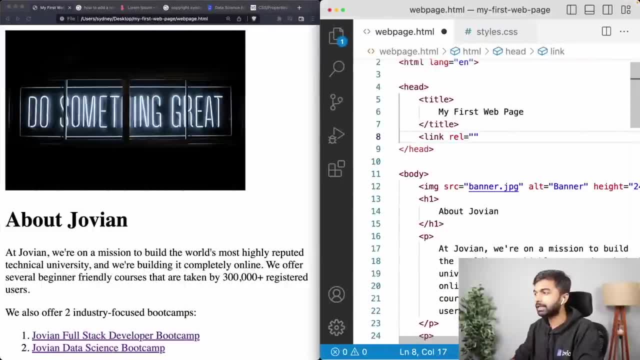 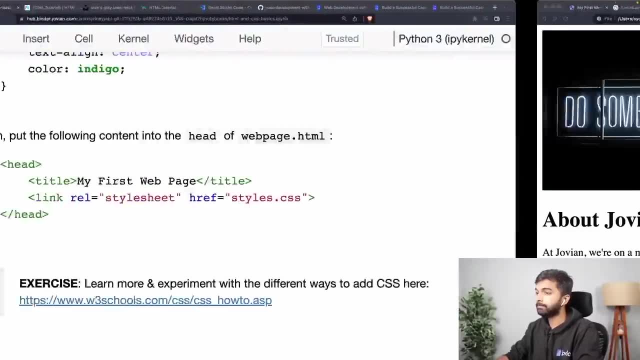 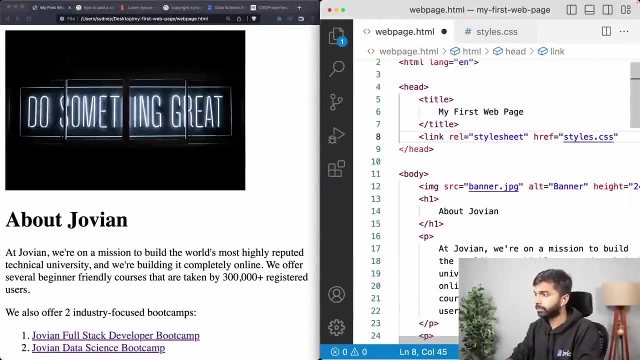 You basically, you basically specify the style sheet, Specify what is the relevance of this link to this page. So, style sheet, or what is the relation of this link to this page, style sheet, and then you say href equal to styles, dot CSS. Okay, 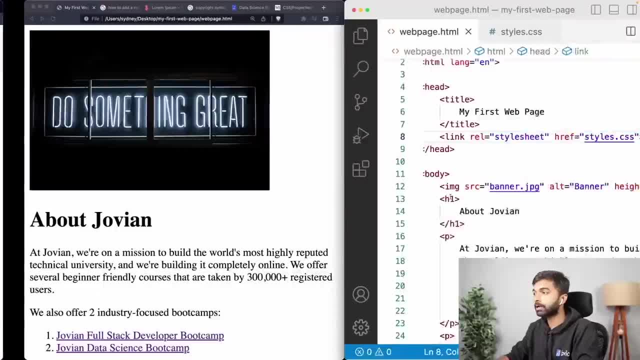 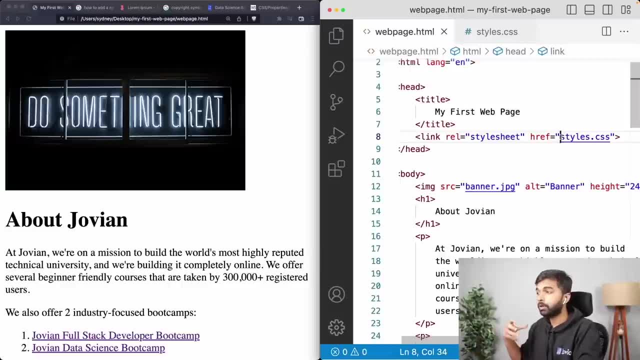 And that's it. And again, you don't need a closing tag. This is a self closing tag. So there are a lot of self closing tags in HTML. Now this href can be a CSS file that is sitting right next to your web page. 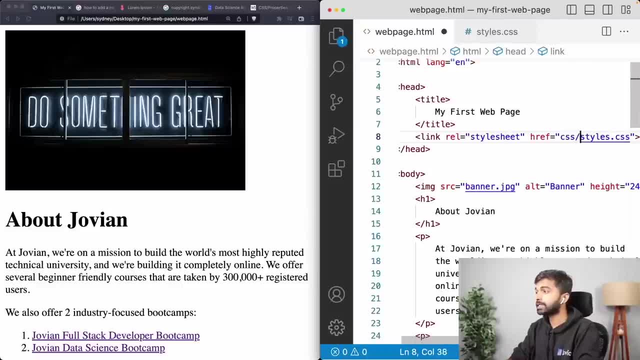 Or it could be in a sub folder. let's say it was in a folder called CSS, then you could put it under CSS slash styles dot CSS. Or you could also specify something on the internet. So that is what is done typically with frameworks like bootstrap. somebody has put up a bunch. 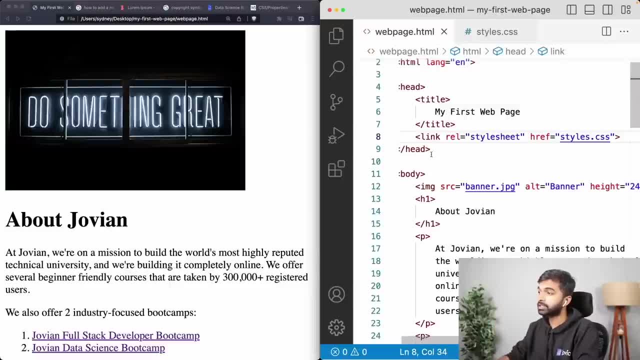 of styles on the internet and we simply include it, link it to our page using the link tag. And notice that the link tag is different from the a tag, which is the anchor tag, which is used to add links on the web page. the link tag is used to simply link style sheets. 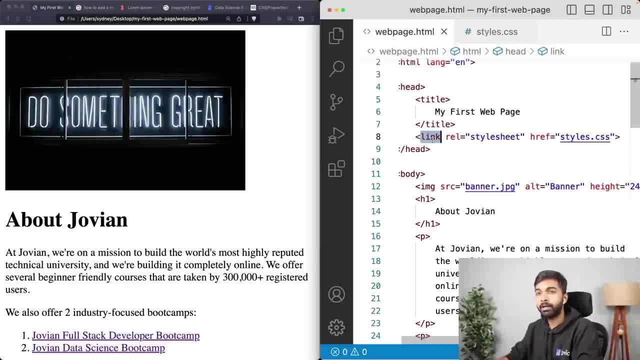 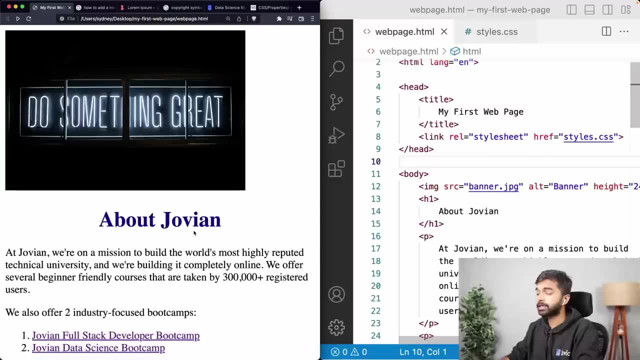 That's a bit confusing The terminology because of how HTML evolved, but that's what it is. Okay, So now we have link rel equals style sheet, styles dot, CSS. Let's reload the page And once again. this is now back to the center and it has the deep blue color. 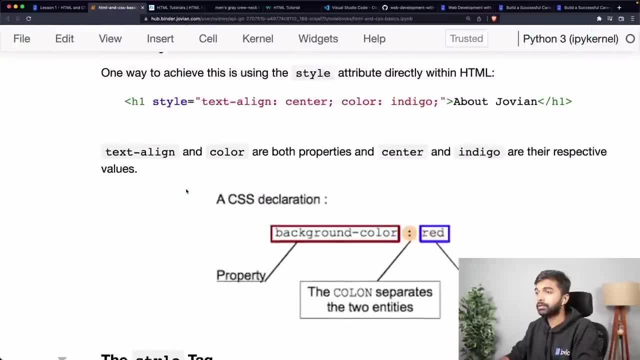 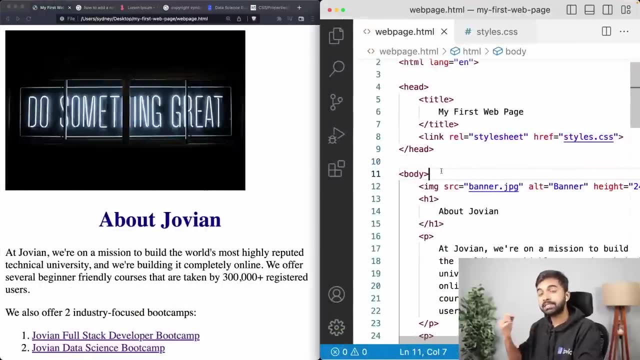 Okay. So those are the three ways in which you add CSS. You have the style attribute, you have the style tag and then you have CSS files. Now, one thing I want to mention is CSS stands for cascading style sheets and inline styles. 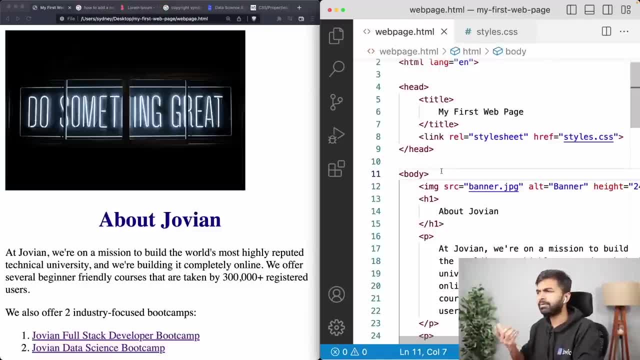 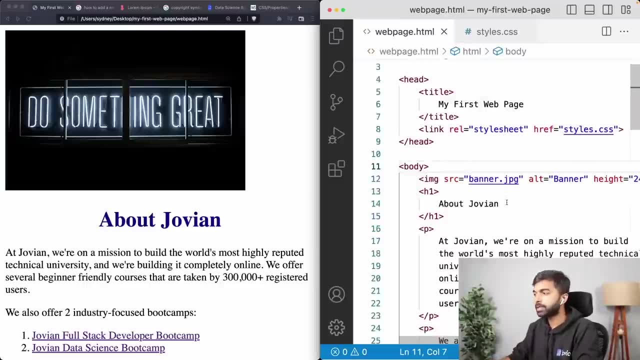 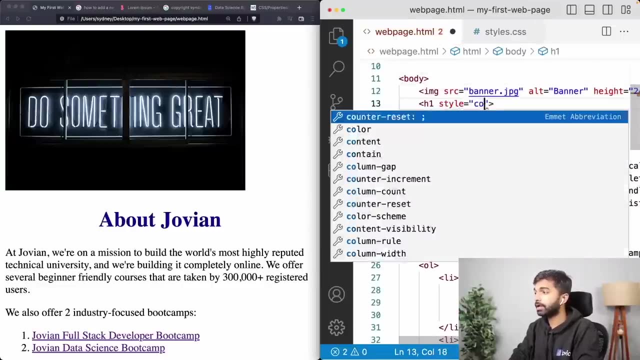 take precedence over style tags and styles. Style tags, I believe, take precedence over the external, external files, And there are also other ways in which precedence is decided. So, for example, like if I went in here and I added a style tag, I did a style attribute. 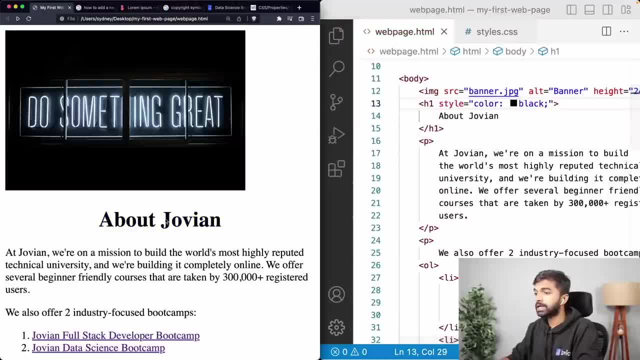 and I changed the color to black again. you will notice that even though the style start CSS file says color dark blue, because I've specified the style explicitly on the H1 tag that takes precedence And that is going to apply the black color to it. 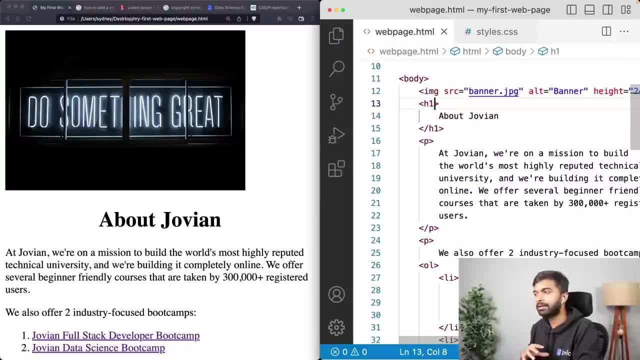 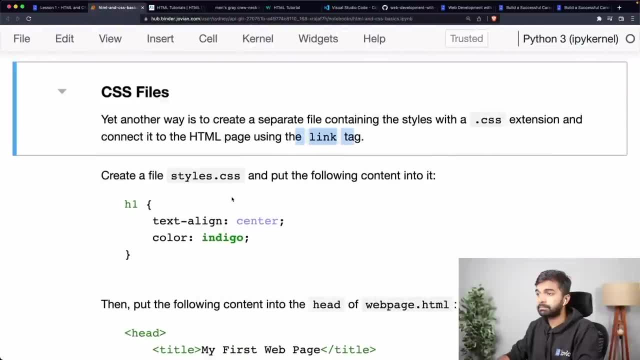 Okay, so keep that in mind. This can be sometimes confusing And, generally speaking, keep things as simple as possible so that you don't run into all these issues. Okay, so, now that we have done we've added CSS, let's maybe look at what are some other. 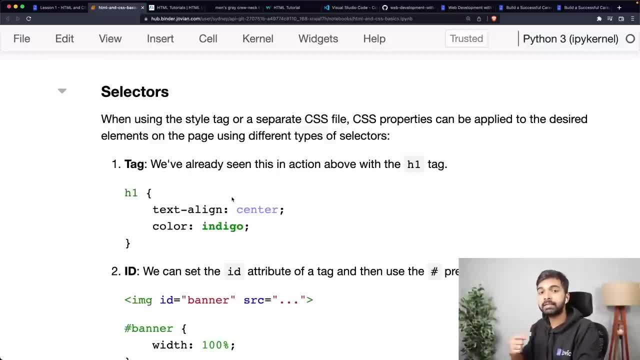 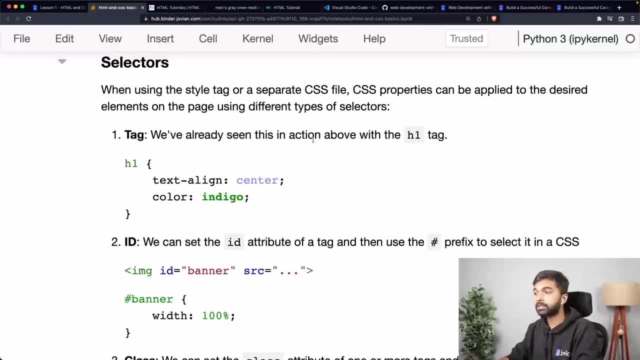 ways in which we can select specific elements and then apply styles to them. So, when using the style tag or a separate CSS file, CSS properties can be applied to multiple desired elements on the page using three types of selectors. One is the tag selector. 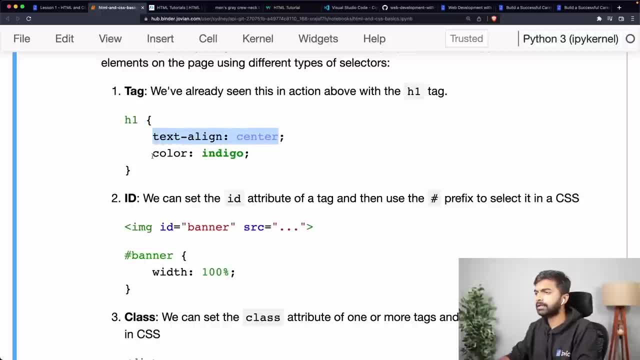 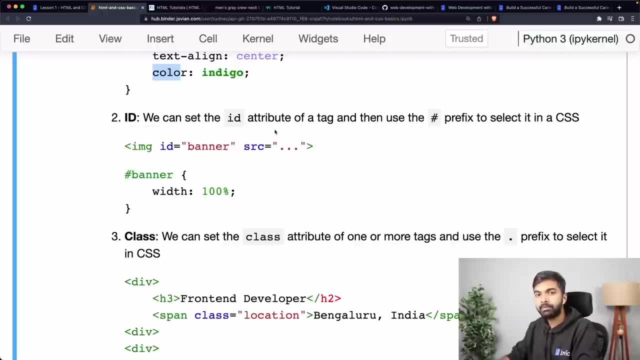 This is something that we've already seen. for example, we've done this text line center and color deep blue or dark blue for the H1 tag. The second is the ID attribute. So typically, what you can do is you can set the ID attribute for a particular tag and 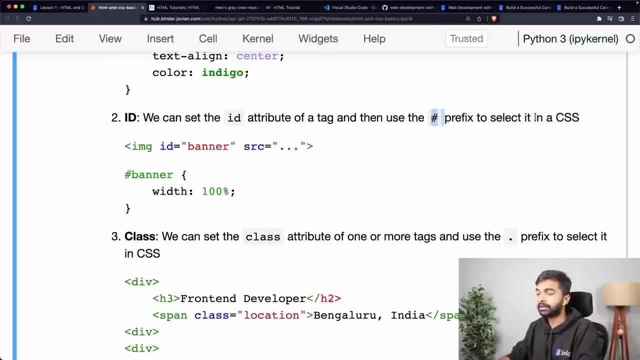 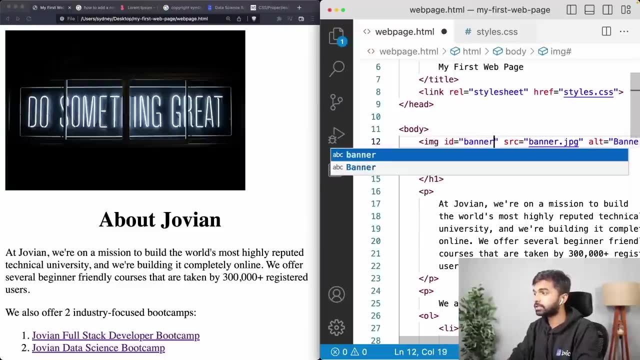 then use the hash prefix within CSS to select it. Okay, so I can do this. I can add an ID for this banner: dot jpg image. So I can just say: ID equals banner And generally, as we go through this process, we're going to see that the tag selector is. 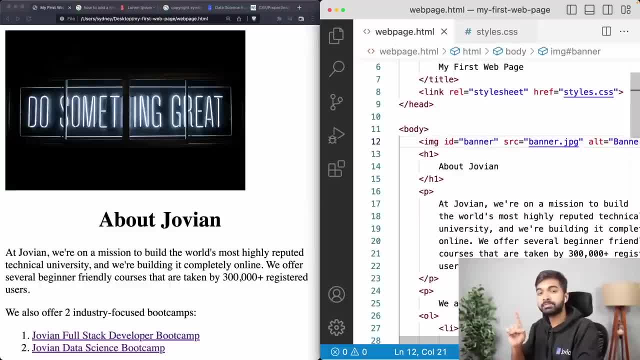 going to be selected. So as a rule, there should be only one element with a specific ID on a page. you can have multiple and the browser won't complain, But just as a rule, semantically speaking, you should have one element with a particular. 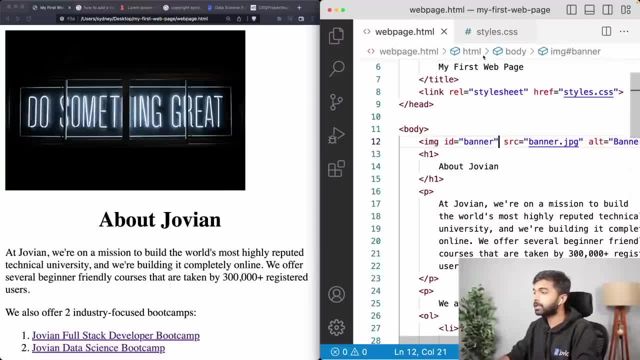 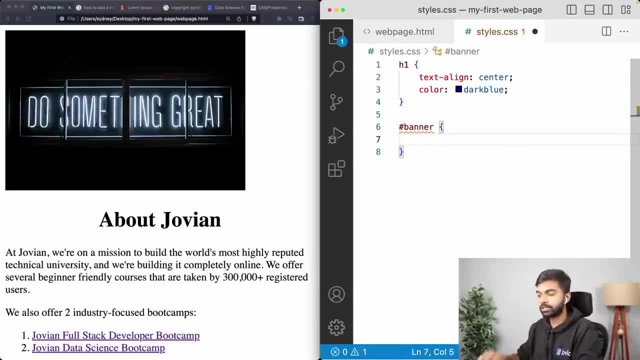 ID on a page. Okay, so ID should be a unique identifier. So now we have banner And now we can select the banner element. Now, if I said IMG, that would apply to all the images on the page. right, If I said IMG, that would apply to all images on the page. but now I only want to apply. 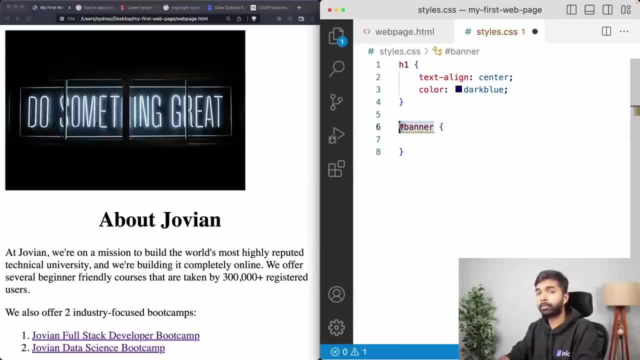 to the tag which has the ID banner, And that is why I have I have this hash or pound character, And now I can set something like width 100%, And now you can see that this image has a width of 100%, 100 width. 100% simply means 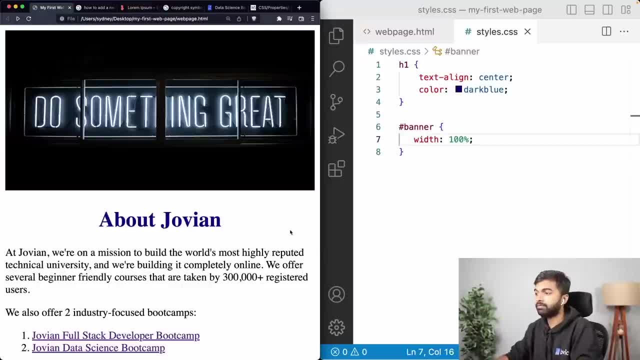 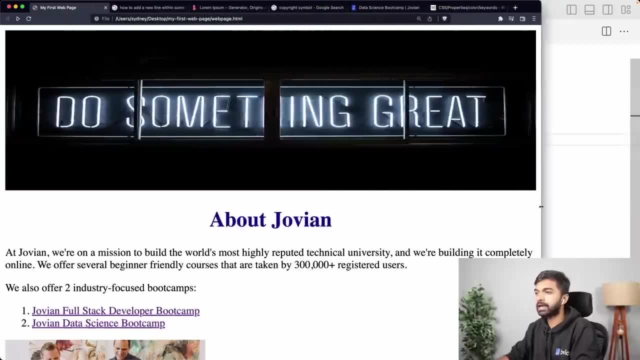 occupy the entire space available horizontally. Even if we resize the page, you can see that this image automatically resizes. Of course there is an issue here that this image is getting stretched. we'll fix the stretch in just a bit, But at the very least we are able to. 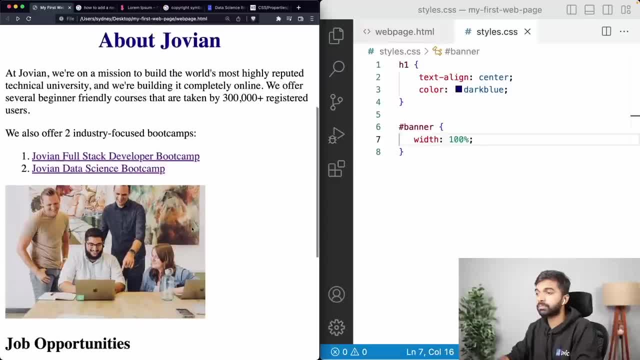 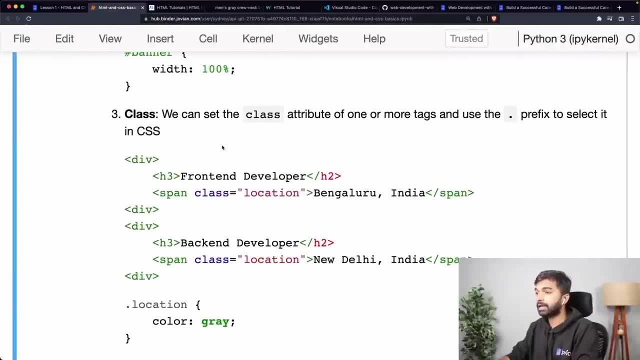 Apply the width of 100% to just the specific image and not to this image. So that is the second way to select an HTML tag and apply some CSS styles to it. Then the third way to select an HTML tag is using a class. 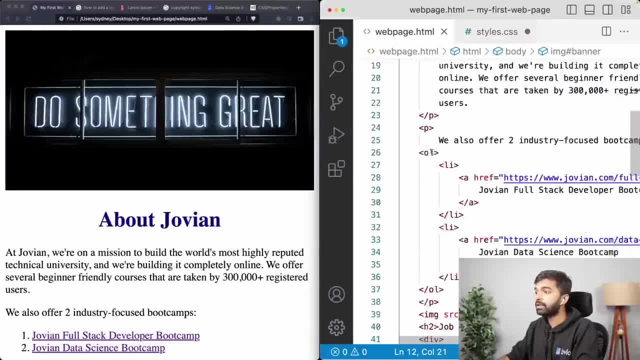 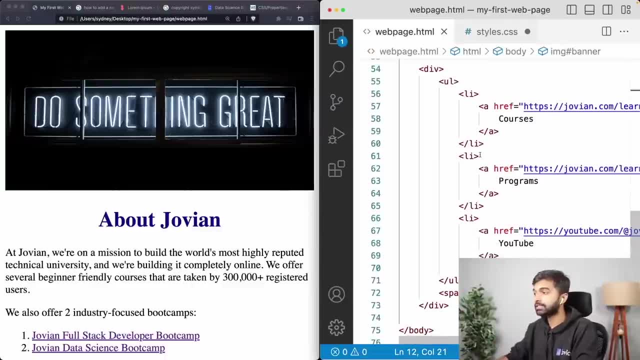 Now sometimes what you might have is a several tags which you want to style at once, And all these tags have to be styled using the same set of styles. So here is an example. Let's say I add location. Let's say I add here: 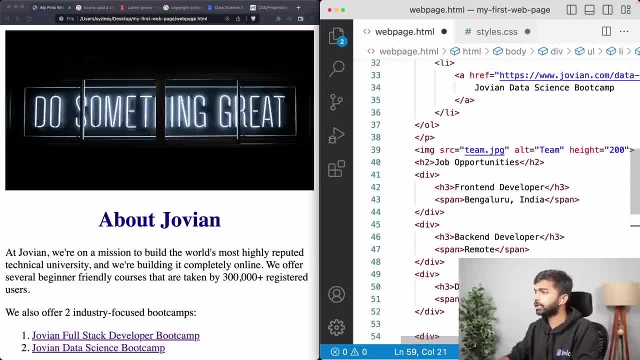 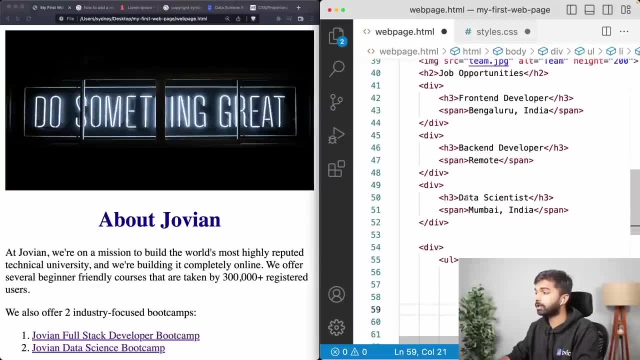 No, I have location somewhere here. Let's say, I look at the location here. Yeah, so I have locations here. I have location for the front end developer role. I have location for the remote developer role- I have located- or the back end developer role and the data scientist role. 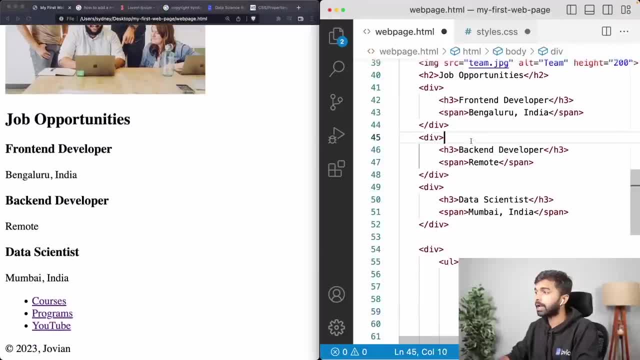 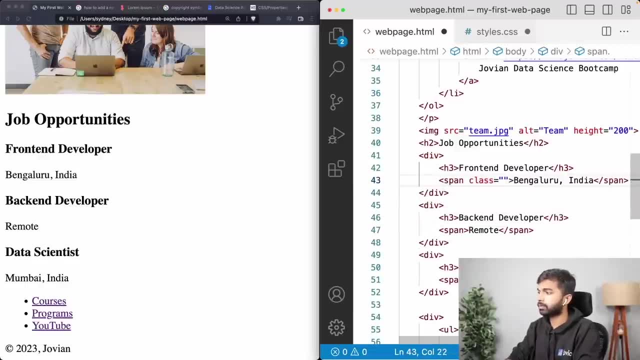 Let's say I want to make the color of the location gray, So I can do this, I can say span and I can say class equals location. Okay, and let me go in and let me add that here as well: And class equals location, and class equals location. 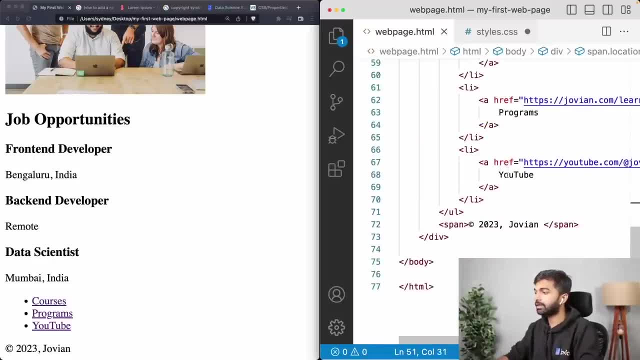 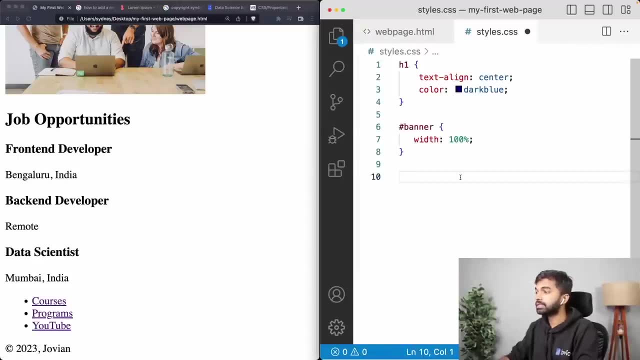 So there may be many spans on the page- you can see that there is a span right here at the very bottom as well- But these three particular spans have the class location. And now I can apply some styles to specifically these three spans by using dot location. 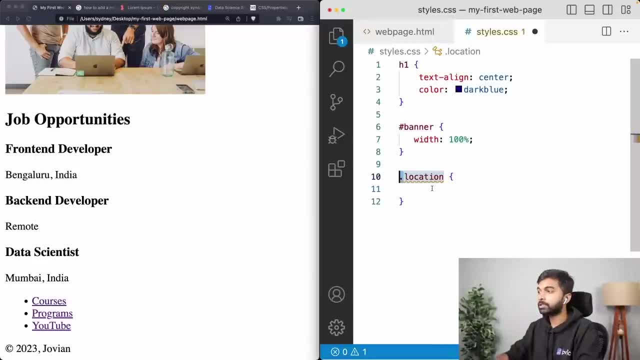 So I can say dot location. dot is used to indicate a class. you can either select a tag where you don't need any prefix, or you can select an ID which is hash, or you can select using a dot which is a class. And now I can say color gray. okay, and let me reload the page. 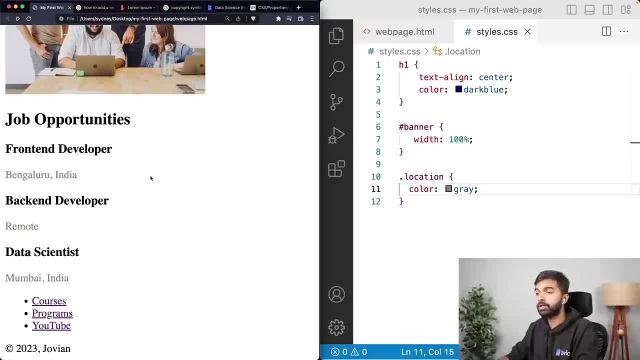 And now you can see, here we have Bengaluru, India, remote- and Mumbai, India. So this is applied, this color is applied specifically to these specific sections. Okay, Now you might ask: okay, how do I know when I should use color, when I should use text? 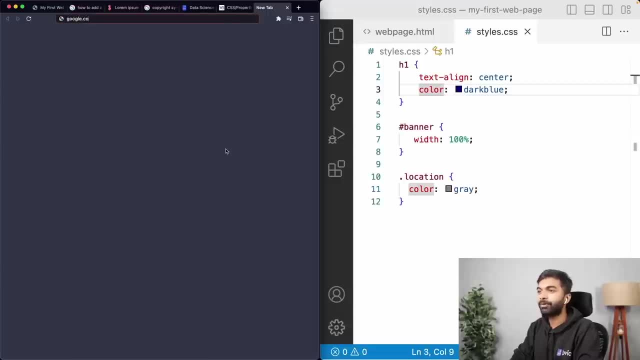 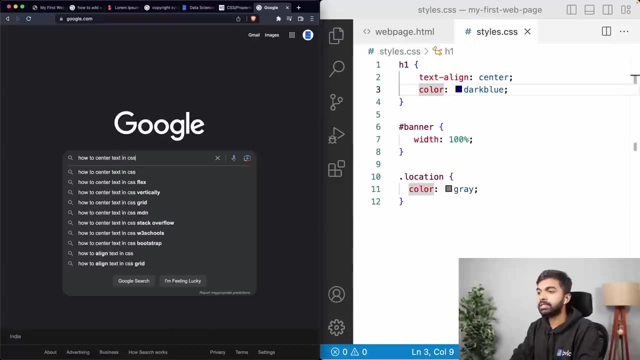 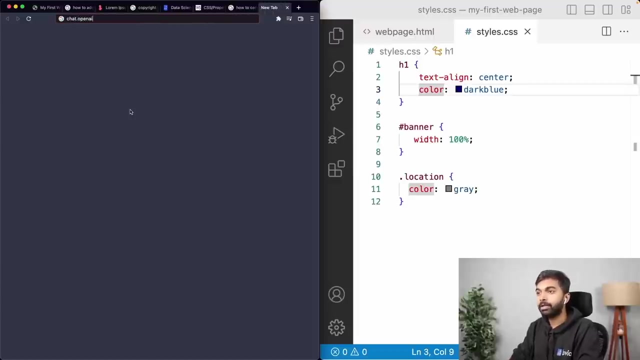 align, when I should use what? the simplest way is to just go on googlecom and search, Okay, How to center X Text In CSS And you can say it uses the text align property. But now we also have tools like chat, GPT, where you don't actually have to go and search. 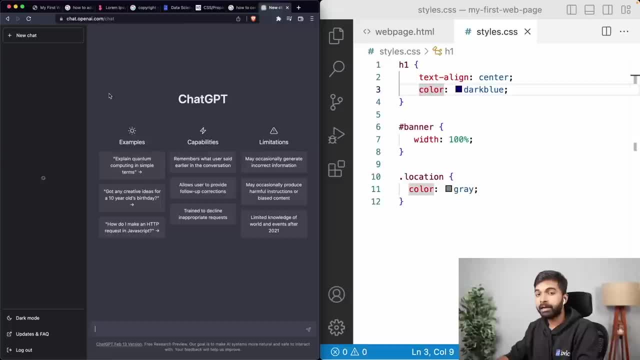 this on Google and browse various web pages, So this is something that I've been using a lot these days. you can see that I have a bunch of conversations here already with chat GPT regarding HTML, but you can just go into chat GPT or chatopenaicom and you can search out to center text in CSS. okay. 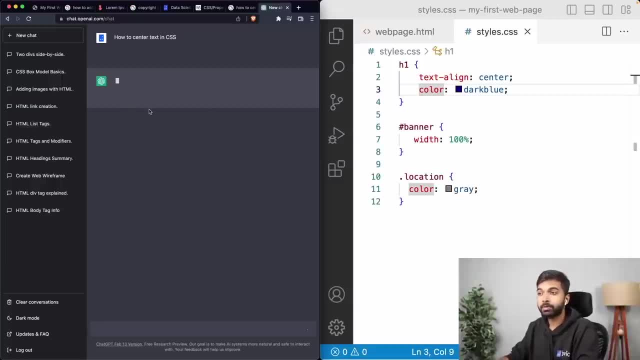 And it is going to tell you that it's going to come up with an answer for that and it's maybe also going to come up with an example, and you can ask it some follow up questions as well. Okay, Let's give it a second. 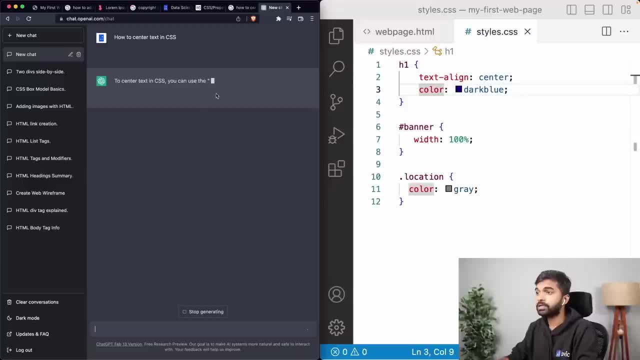 Maybe it will come up with. Yeah, to send a text in CSS, you can use the text align property and set its value to center. Okay, and it's showing you an example as well. Okay, So, let's see. Okay, So, let's see. 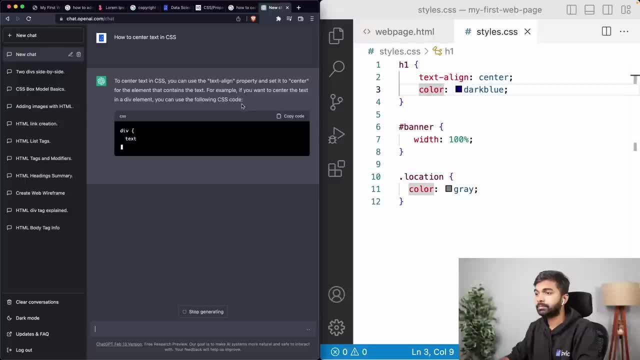 So let's see Okay. So let's see Okay, Let's see All right, and that's it. So you, This is great, It works really well. it doesn't always give you the right answer, But you could ask it a couple of things and you can try it out. 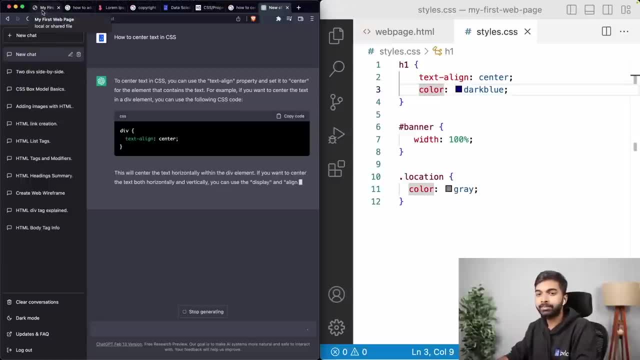 It's a good starting point, whenever you face an issue, to go ahead and ask in chat GPT. In fact, I'll encourage you: some of the questions you've been posting on zoom, try posting them to chat GPT and you might be surprised at how well it can answer these questions. 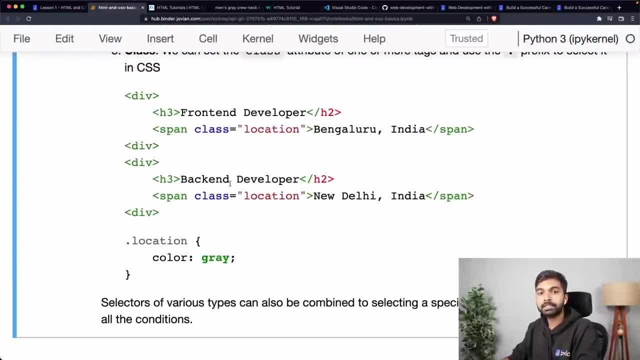 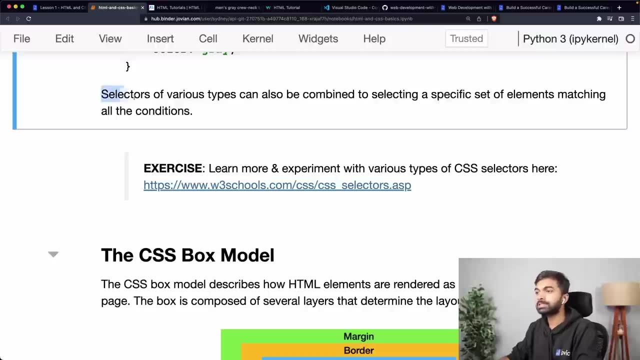 Okay, so that is about the different ways in which you can select things. Now I encourage you to learn more and experiment with various types of CSS selectors. What you can also do is you can combine selectors of various types to select a specific set. 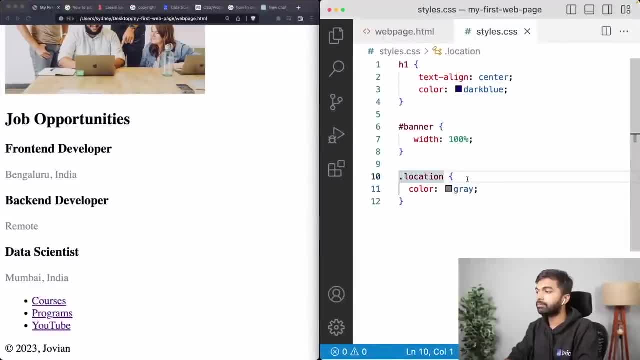 of elements that match all the conditions. For example, let's say you have certain divs with the class location and you have certain spans with the class location and you only want to apply these settings to the span with the class location. then you can say span dot location. 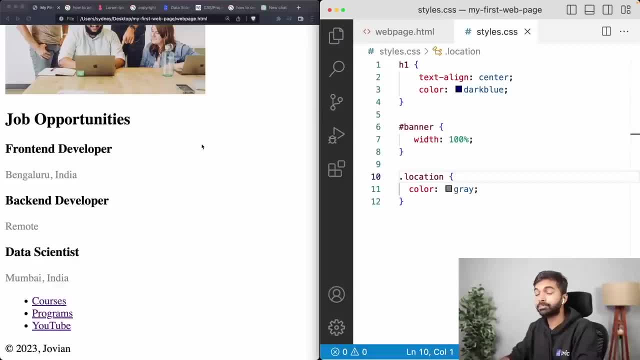 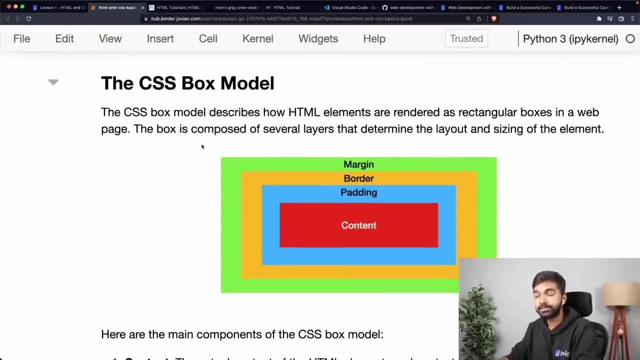 And I believe that is going to expand our location And I believe that is going to just select the spans which are the class dot location. Now, the next thing I want to tell you, before we go ahead and actually style the rest of the page, is the CSS box model. 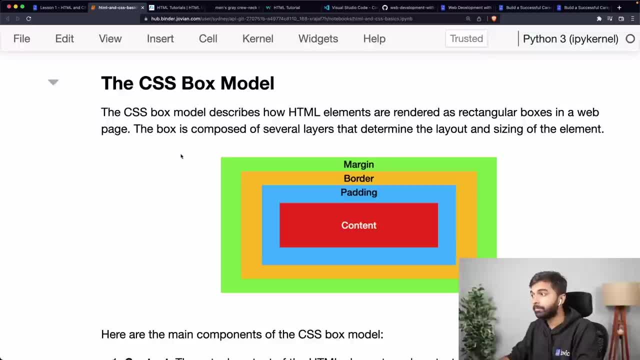 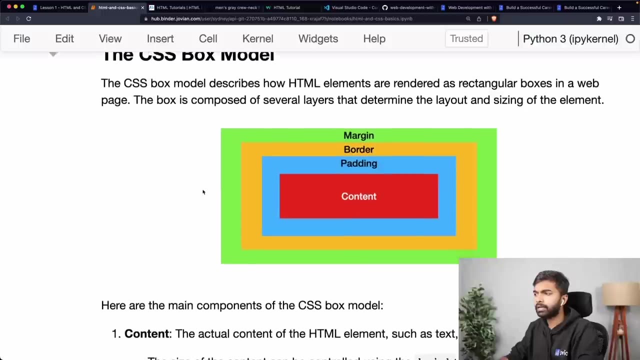 The CSS box model describes how HTML elements are rendered as rectangular boxes in a web page, And the box for any HTML element is composed of several layers that determine the layout and the sizing of the element. So let us create. there are a few components to the box model. there is the content. there. 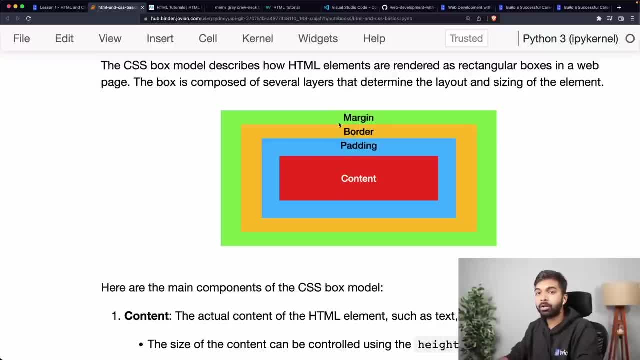 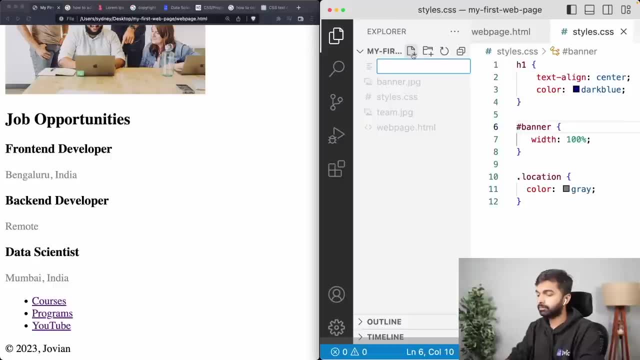 is a padding, there is the border and there is a margin. We are going to understand all of these terms And we'll do that by creating another web page, just so that we can experiment with the box model. I'm going to open up the sidebar here and open up another page called box model dot. 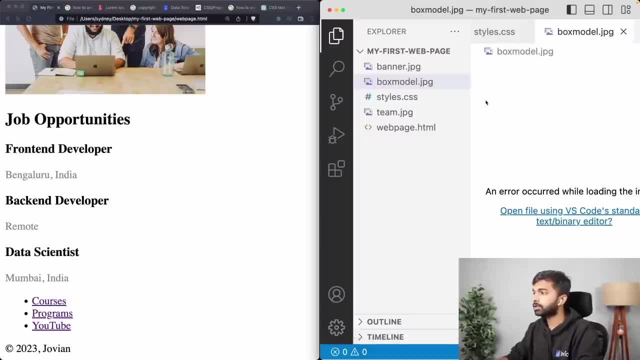 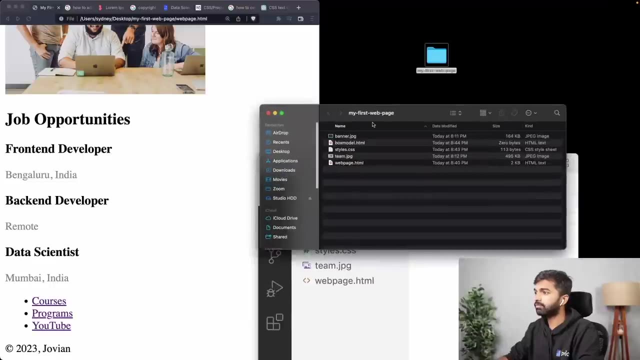 jpg. Okay, there it is box model dot jpg. Oh sorry, Box model dot HTML. let me rename that. Let me create another page called box model dot HTML. Okay, And I can open up box model dot HTML here in my web page. 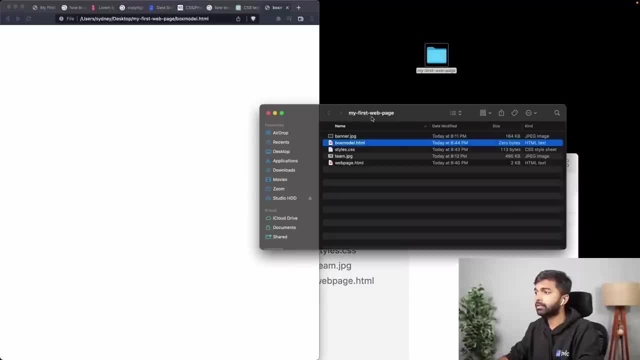 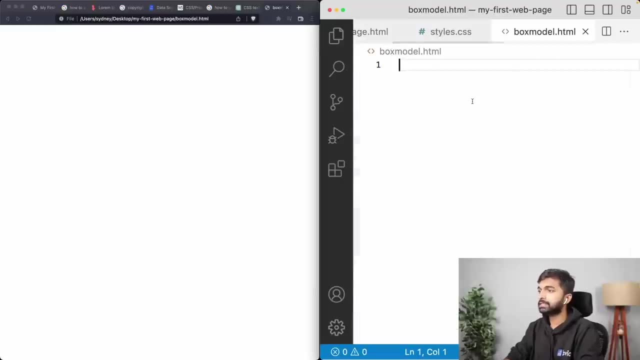 And in my web browser, like that, just double click on it. Now that opens up box model dot HTML for me. And now inside this, let me start putting in some content. So HTML, let me put in the doctype declaration as well. 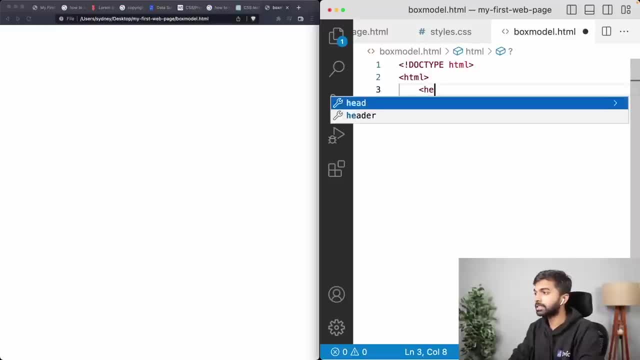 You can see that VS Code auto completes the doctype declaration. It's nice, So let me add head, Let me add a title here, So CSS box model, And let me add the body here And let me add a couple of divs. 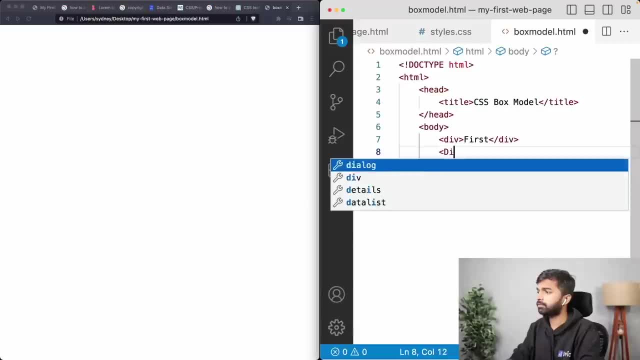 So let me add a div called first, Let me add another div called second, And let me give both of these divs a class each. So let me call this box one. By the way, for class names you can put hyphens in between. 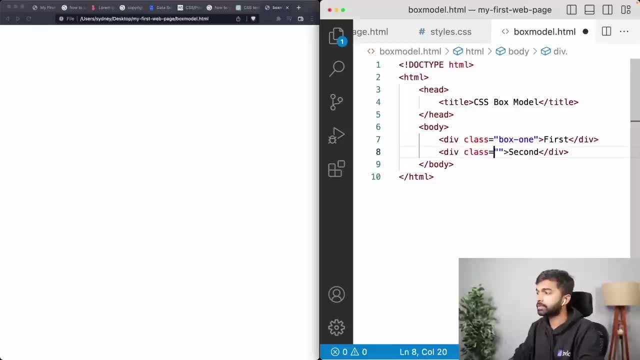 So in CSS, whenever you're using class names or IDs, you can put hyphens. Let me call this box two. Okay, Let's reload that. Let me zoom in a little bit when it is good enough. Yeah, you can see that we have content as we expect. first and second. 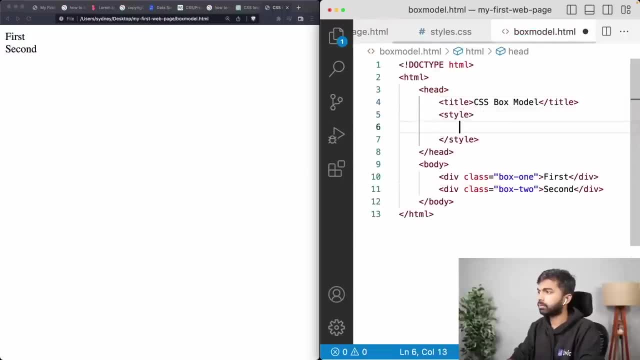 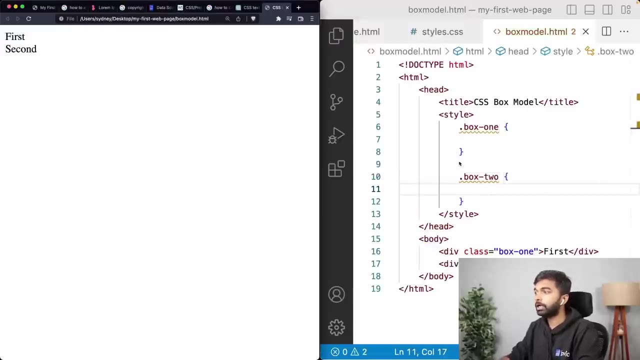 Okay, let me add a style tag here, And for box one I'm going to set some styles, And then for box two I'm going to set some styles. Okay, no change here so far. Now, the first thing I want to point out is: what does the content of a div look like? 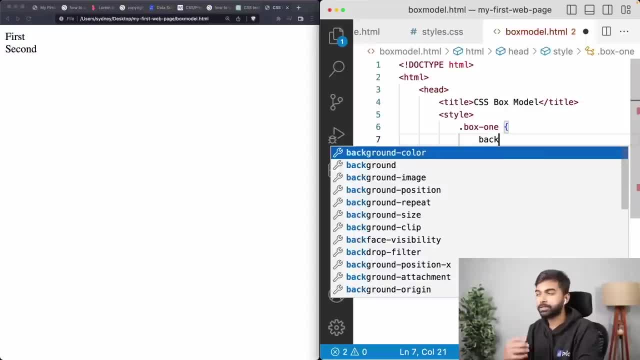 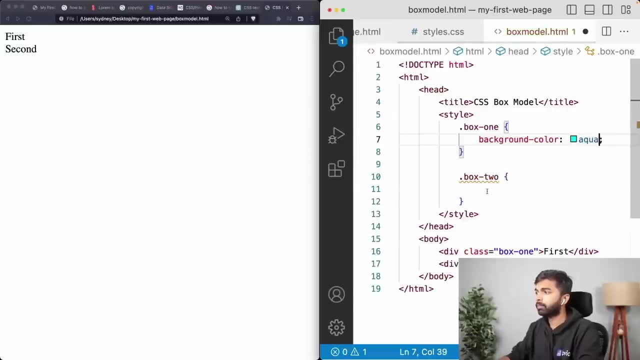 Well, let me add a background color. So the way you add background color is: you just start typing and VS Code shows you. So let me add a background color. Let me add the background color aqua for box one, And let's add a background color. 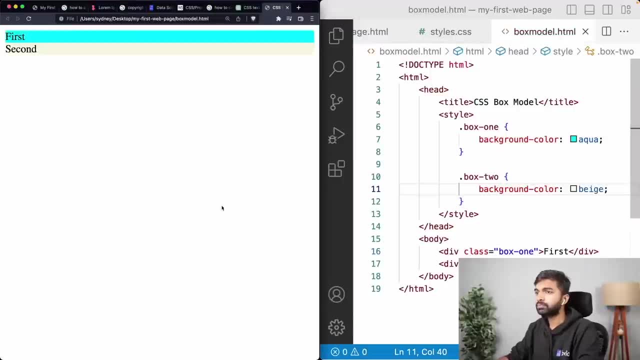 Let's see beige for box two. Let's reload that And now you can see that each of these boxes or each of these divs, and a div is essentially a box which occupies the full width of the page. mostly, each of these boxes have a background. 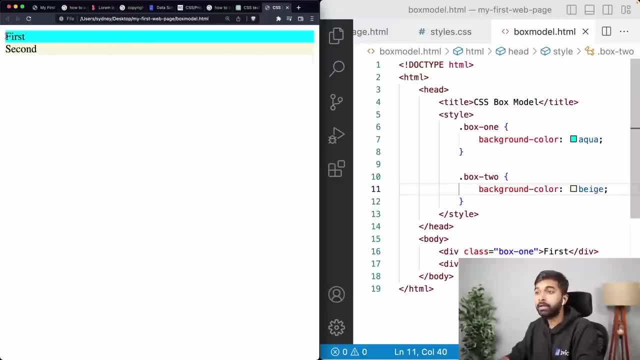 color. One has a background color aqua and one has a background color beige. okay, this first notice that the content of the of the box occupies the entire width by default. when you create a div, you can see that there is some empty white space around. that is because 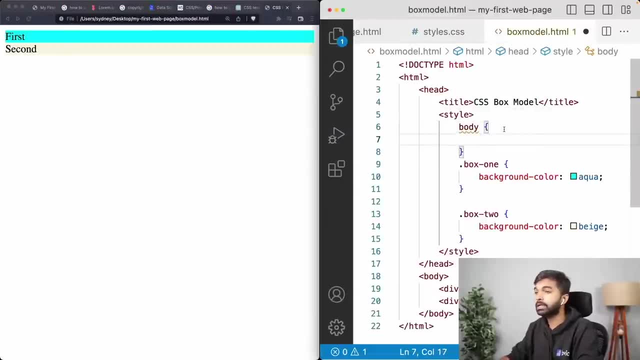 the body. the body tag, which is the outermost tag on the page, contains some margin and padding, which I'm going to, or some internal spacing, which I'm going to just set to zero for now. We'll understand these terms- margin and padding- in just a second. 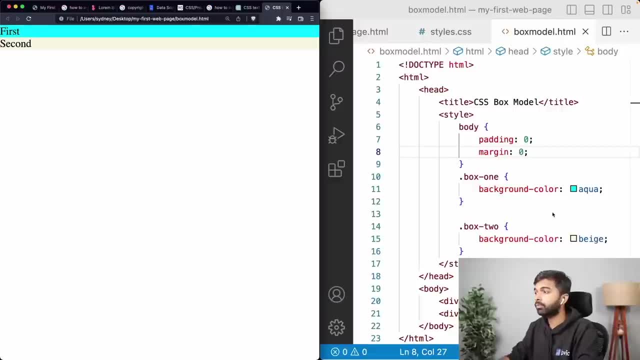 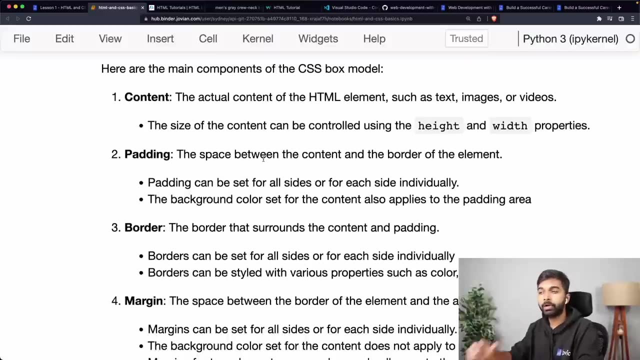 Yeah, So now you can see we have first and second And second. we have a box one which is first and box two which is second. So you have the actual content, which is the innermost component of the box, And right now our boxes just have content, they don't have anything else. no, no border. 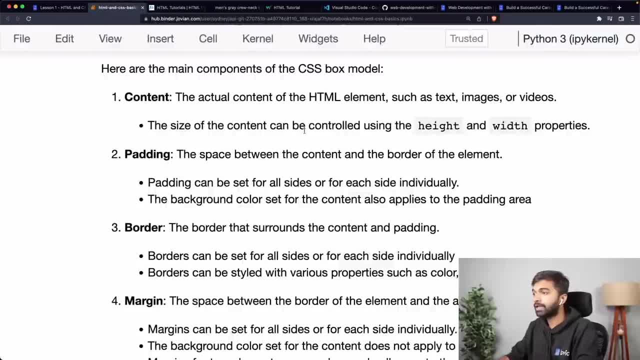 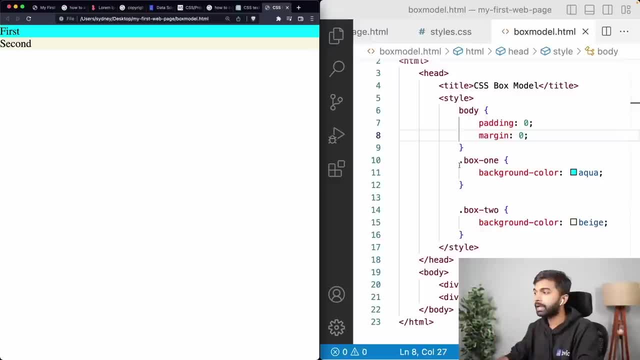 margin padding nothing. Now the content itself can be controlled using the height and the width properties. Of course, if you put in a lot of content, the height will automatically expand. But I can also set the height specifically. I can say this: should have the height 240. 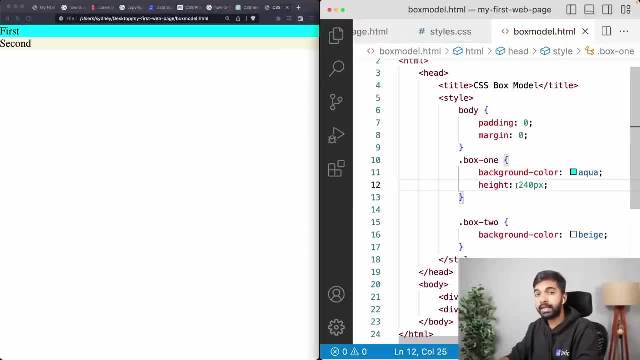 px. And this is how you specify lengths in a CSS: you specify a number and then you specify px. Now you can also specify in inches, you can also specify in percentages and all, But in the current case, I'm just going to use px. okay, 240 seems too big. 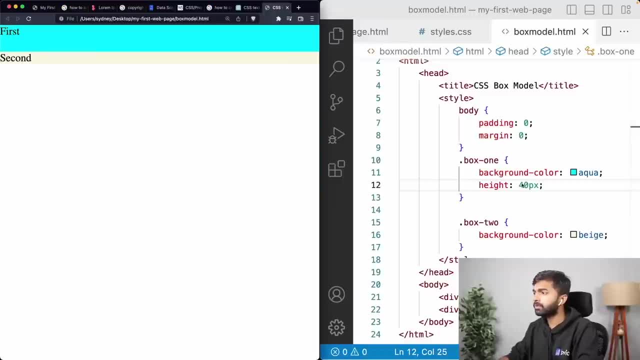 Let me just set it to 40 px right now. Yeah, Now we've set the height to maybe 80 px. Okay, so now we've set the height of the first container, or the first box, to 80 px, And let's set the height of the second box as well. 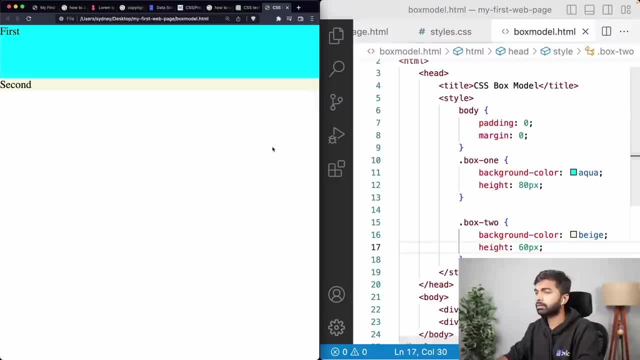 I'd X tp x. the height of the second box is said as well. so far, we just are boxers, just have a content, Nothing special. Now, the next thing that we can add is something called a padding. Now, the padding is the space around the content. 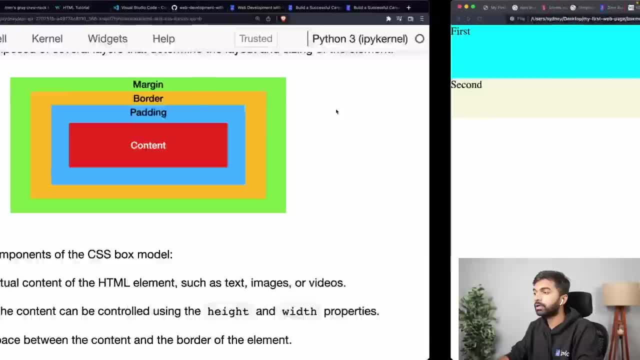 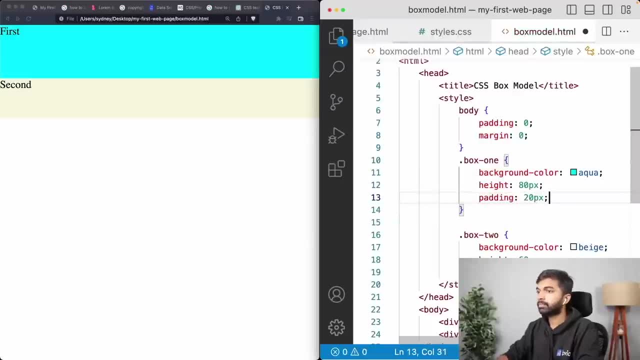 So you have the content and then you have padding, which is a space around the content. Okay, so let me add adding 20px and reload the page. Okay, you can see that we have this box first and the content itself is of height 80, but then around it. 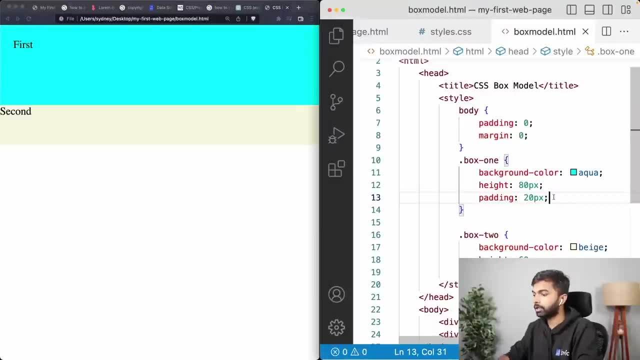 there is this additional space of 20 px. okay, you can. you can, by the way, you can just comment out something. or you can disable some css property simply by putting it under these: uh, slash star commands, um, and you can do this using the command slash. okay, command plus, slash is going to comment. 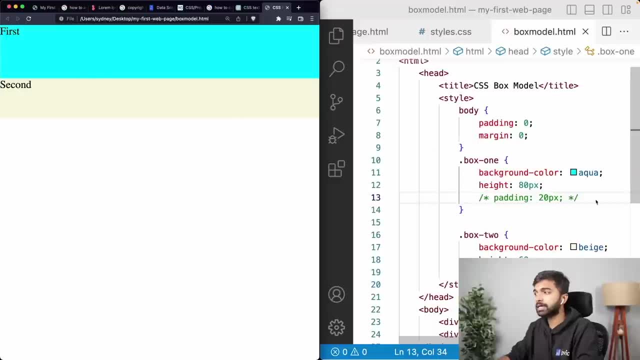 something out. you can see without the padding it this is the size and then with the padding, this is the size and clearly it is added more it. we have added some space before the on the left and also, you'll notice, on the right as well if you try to actually do something with it. 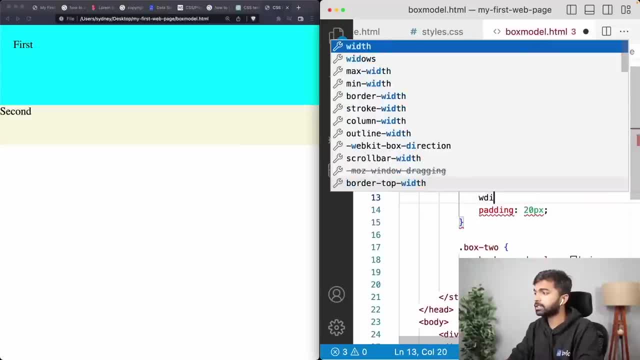 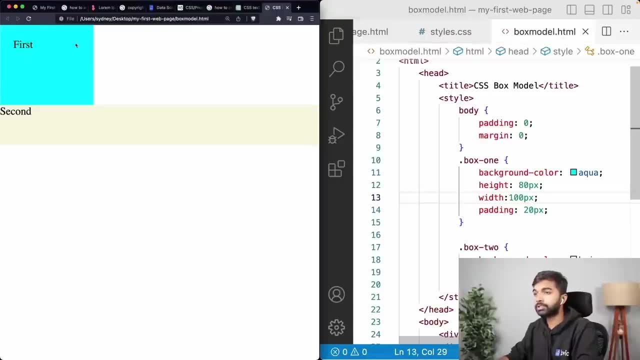 okay. so let's say we set a width. i can also set a width here with 100 px. again, you can see that this is the structure, or this is the content of the box. without padding, this is what it looks like, and with padding it is added around the content. so padding is space around the content. but the key thing, 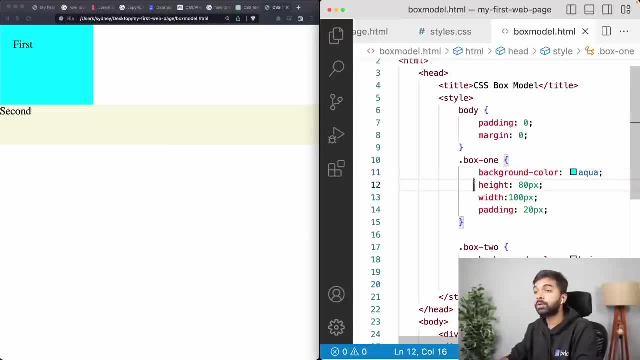 about padding. is that the background color or the background image or whatever? also applies to the padding? okay, now, next thing that you can do is you can set a border. you can. you can set a border. you can set a border of, let's say, one pixel and let's just reload. nothing happens. 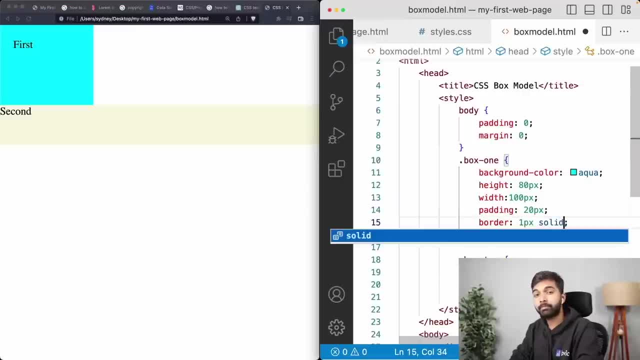 because when you're setting a border, you need to specify not just the border, uh width. you can set the border width of the box. at the same time, you also need to specify what kind of border you need and the. typically, the border that you need is like a line border, which is 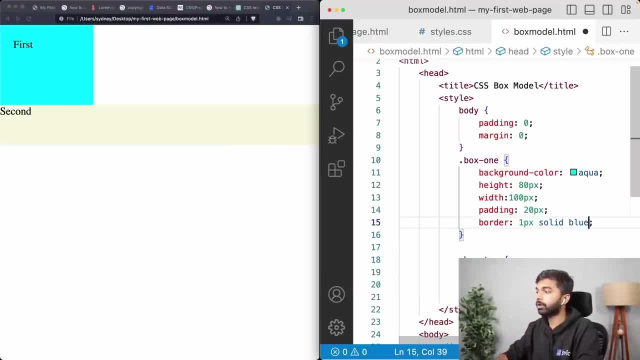 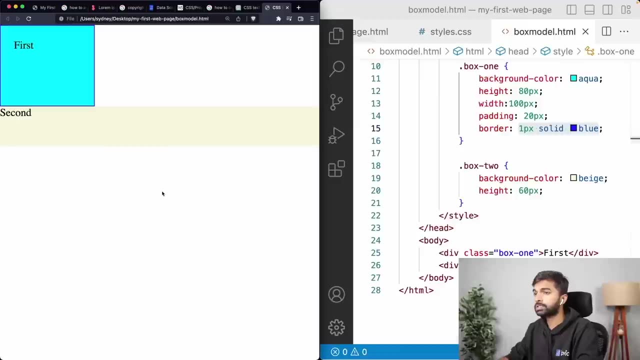 solid, and you also need to specify what is the color of the border. okay, so 1px solid, blue. that is what i'm setting as the border of the of the of the box. okay, so now you can see that outside of the padding, a border has been added which is blue in color. let's make that 10 pixels. 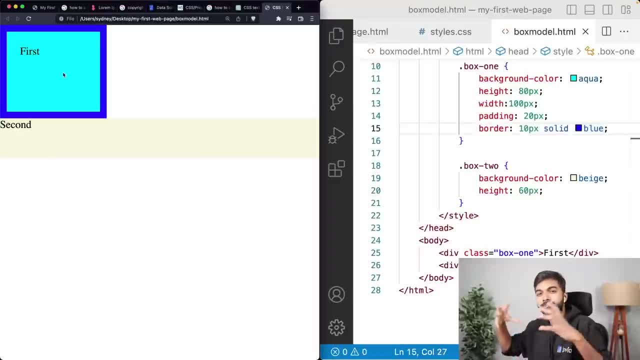 so now we have a 10 pixel border and you can see once again the size of the entire box has grown. So first we have the content and then around the content we have the padding, which is indistinguishable because it has the same background, but it is space. 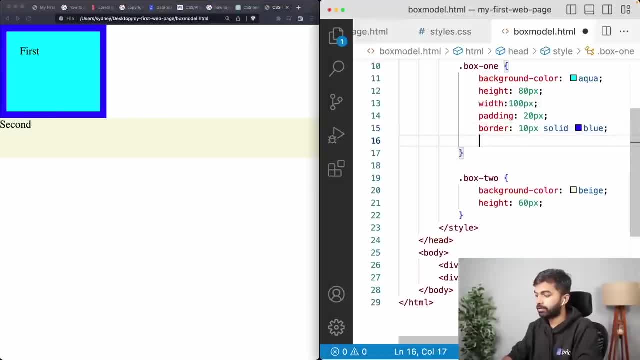 You can clearly see, And then around the padding we have the border. by the way, you can also add a border radius radius here. Let's say you can add a border radius of 20 pixels, and a pixel is simply one point on. 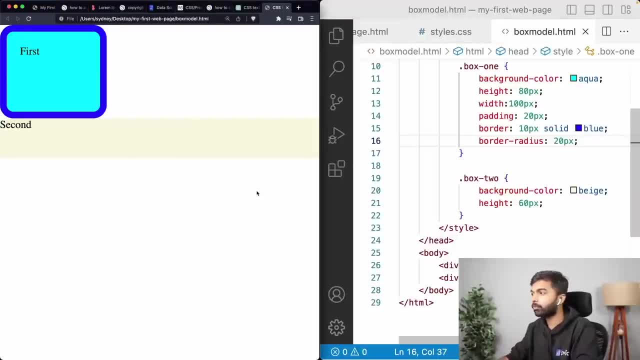 the screen. Okay, And you can. just. you can just play around with the pixel values when you're experimenting and over time you'll get a sense of which what pixel values make sense for the webpage you're working on. Okay, But I'll remove the border radius for now. 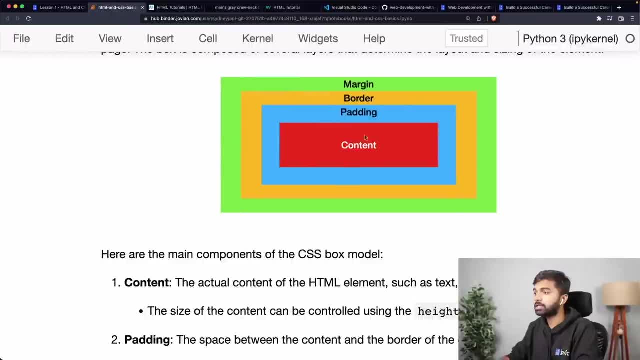 So now we've added a height, we've added a width, we've added a border. So we have the content and then we have the padding, and these two are indistinguishable because they have the same background. Then we have the border, and the border has its own color. 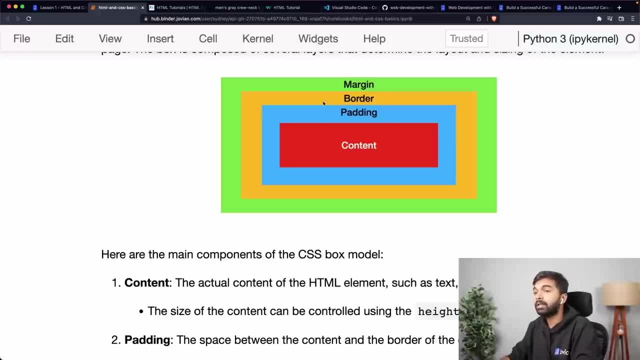 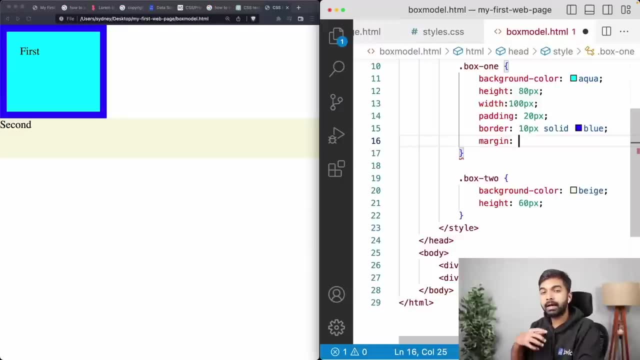 It can match the background, It can be different, but it's going to show up separately. Then you can add some space outside the border as well. Okay, And that is called the margin. So margin and padding are the two most confusing things for when people they're getting started. 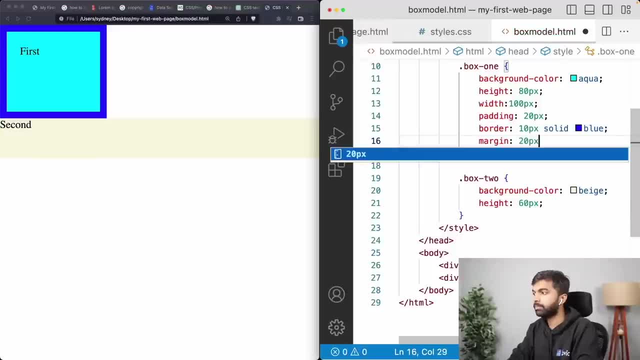 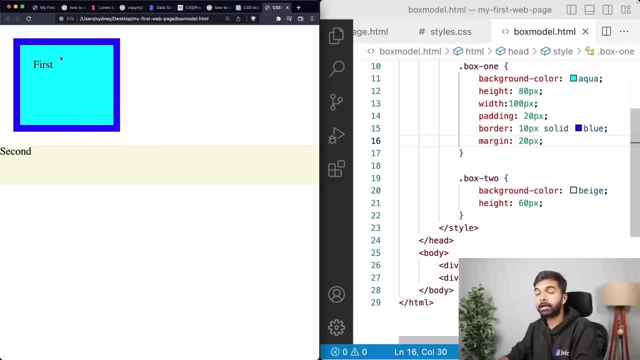 with CSS, So I hope this is going to clarify. So let's say margin 20 PX And when we add a margin of 20 PX, you can see that outside the border, 20 pixels have been added left and right around the entire box. 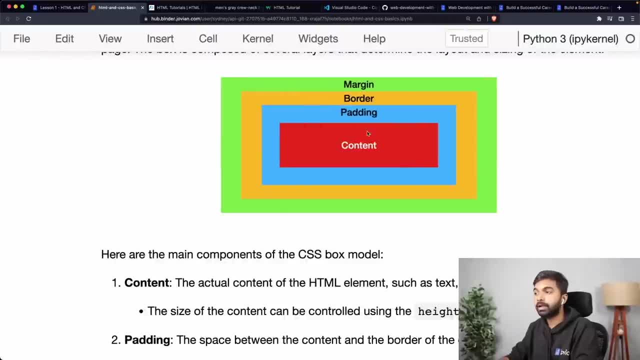 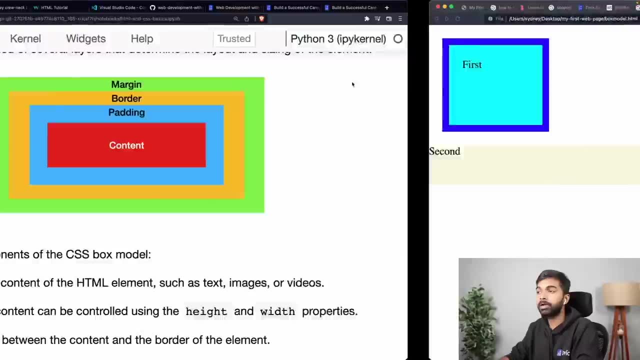 Okay, So the CSS box model basically tells you that you can get some content, then put some padding around it- and that'll have the same background- and add a border around it and then add a margin around it which is going to space it away from the other elements on the page. 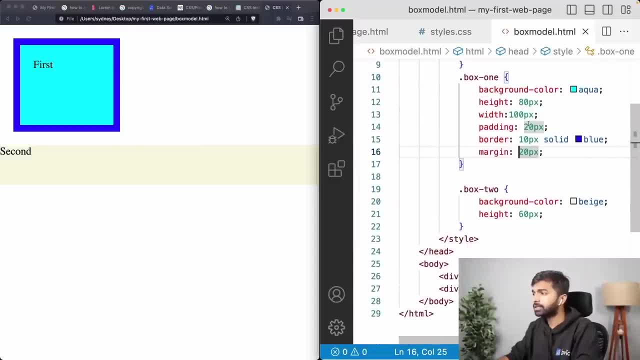 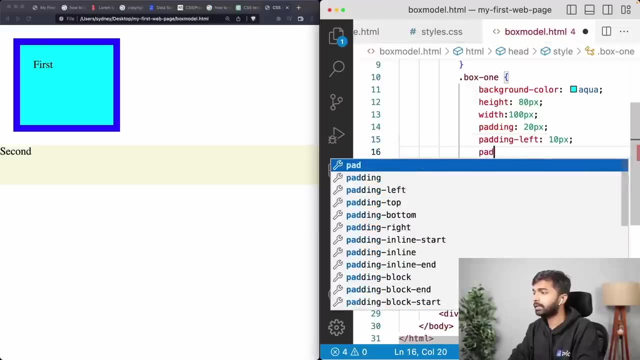 Okay Now. So border and margin, padding and margin- you can actually use a different border side. You can use a different border width or padding width on each side. So, for example, you could say something like this: padding left is 10 PX, padding right- 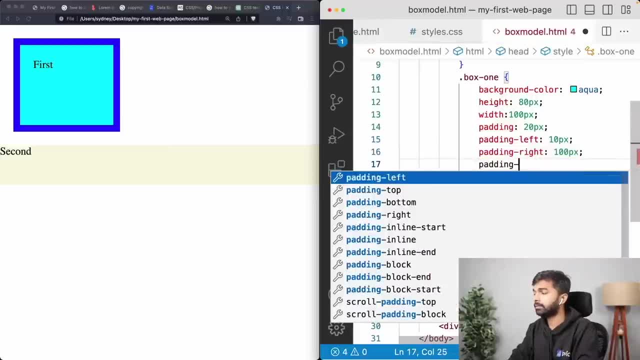 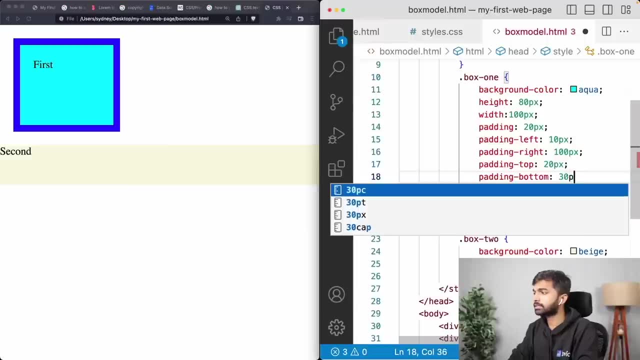 is 100 PX, padding top is 20 PX and padding bottom is 30 PX. Okay, Let's for a second. let's just disable that. I'm just commenting it out. or basically, this is done using command plus slash. Okay. 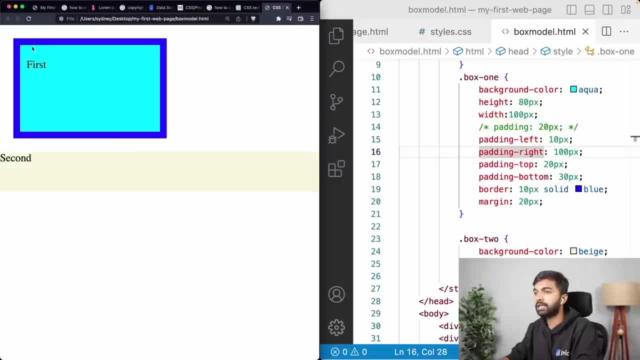 And you can see, now we have some padding here, and then we have some padding here which is, which seems to be higher, And then we are going to have some padding at the bottom as well. You can, you'll be able to see it more accurately if I hide. 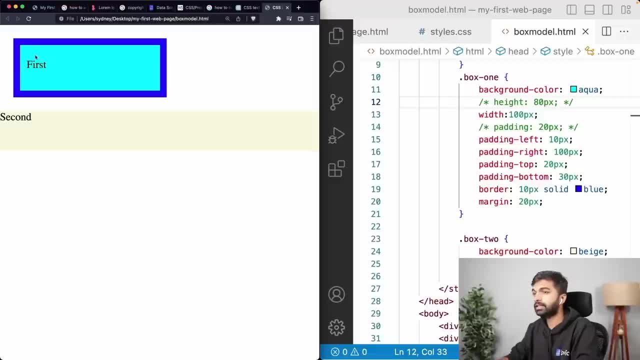 So there's higher padding at the bottom, lowest padding at the left, and then there is some medium padding here, And then there is, of course, a lot of padding here without the right. padding is going to be different. So that is one thing you can do. 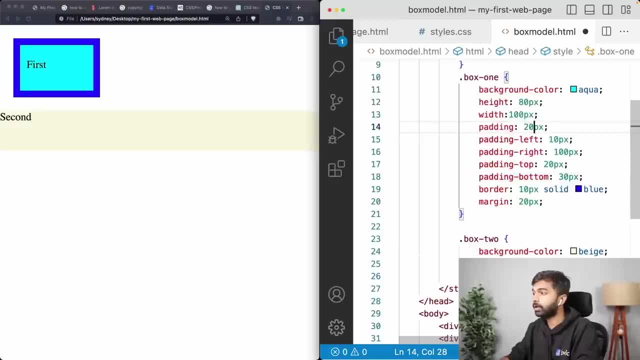 You can actually specify padding properties for each side separately, or you can also just specify for all sides directly here, So you can say: 10 PX, left padding, 100 PX, right padding, 20 PX. Oh, sorry, You have left. 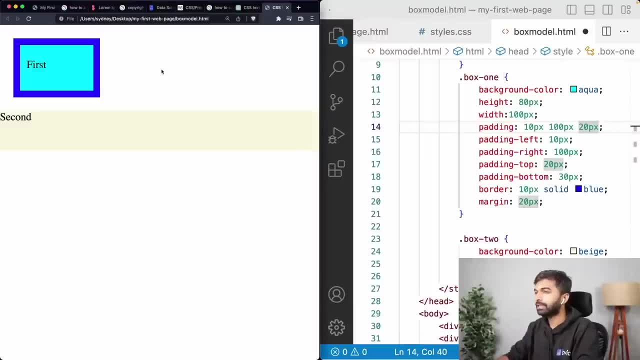 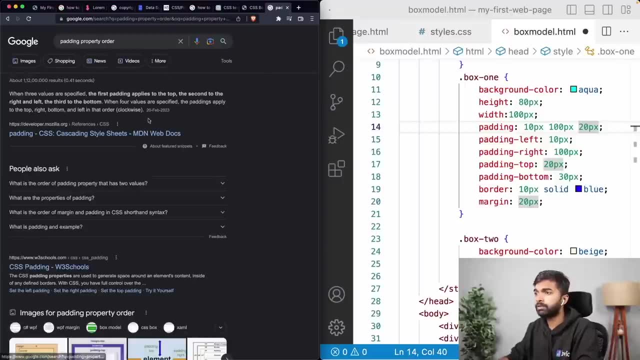 No, I'm not sure. Well, I think you start from the top, you start from the top. So padding property order. Yeah, So the first pair of first padding applies to the top, The second to the right, The second to the right. 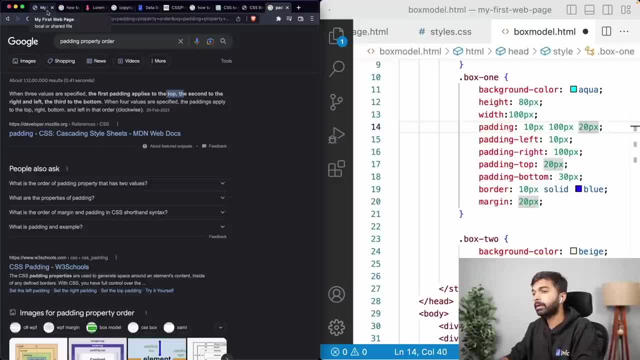 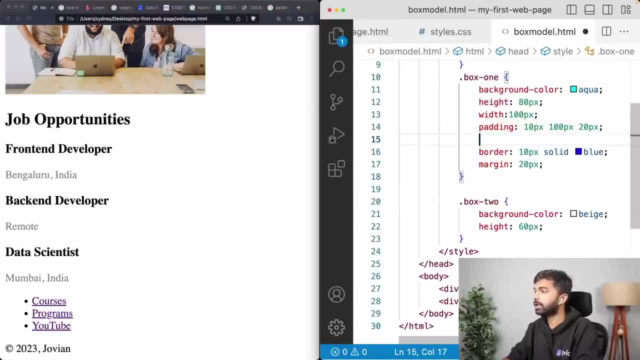 The third to the left and the third to the bottom And then the last one to the left. Okay, So instead of padding, left, left, right bought the top, bottom. you can have padding, and then you can specify what padding you want for the top, what padding you want for the right. 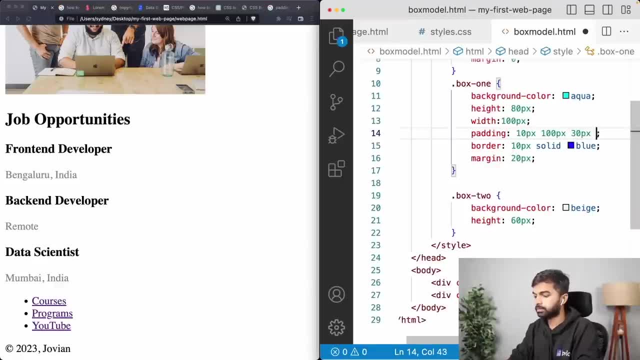 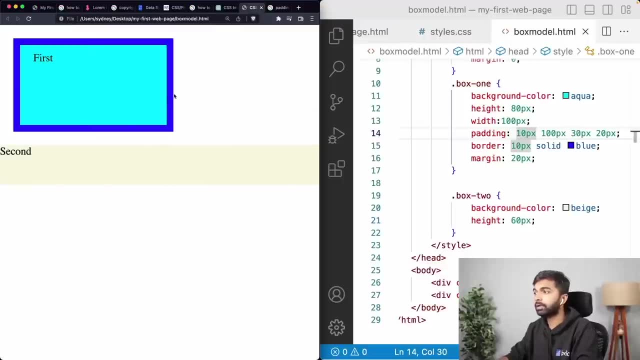 what padding you want for the bottom and what padding you want for the left, or 20 PX? Okay, And that is going to set the padding top right, left, top right, bottom left. Okay, So that is padding top right, bottom left, and similarly you can specify margin separately. 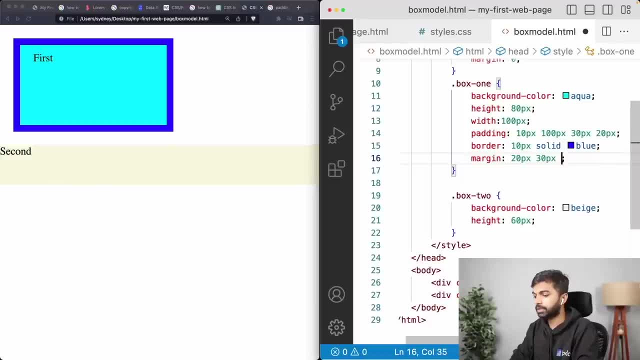 as well. So you can say 20 PX at the top, 30 peaks on the right, 50 PX at the bottom and a hundred PX on the left, And that is our margin applied properly. Okay, Now, one thing you can also do is let's say your top and bottom margins are equal or top. 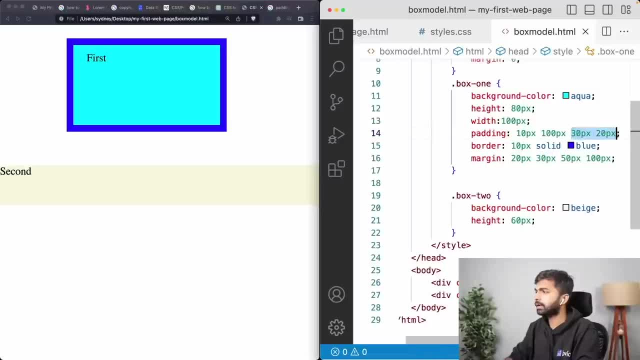 and bottom paddings are equal, Then you can keep them the same. So you can. you can do this. You can say: Margin of padding: 10 PX and a hundred PX, So the 10 is going to get applied to top and bottom and then the hundred peaks is going. 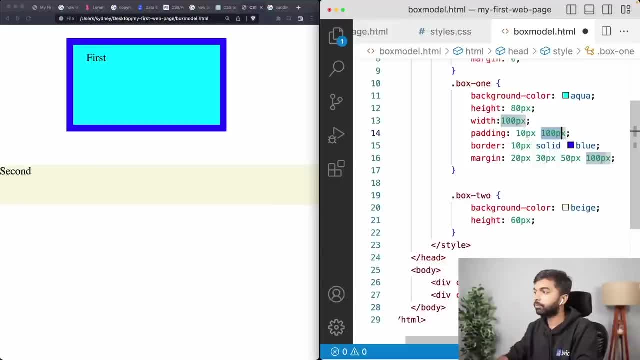 to get applied to left and right. Okay Again, top bottom, left right. If you put just two values, it is going to repeat those two values. Okay, Top bottom, top. top right, left, bottom. clockwise order: top right, left, bottom. 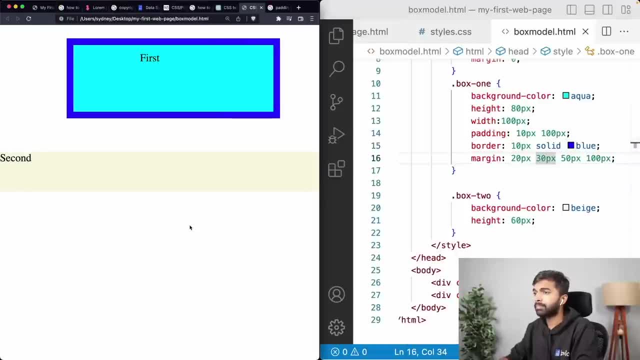 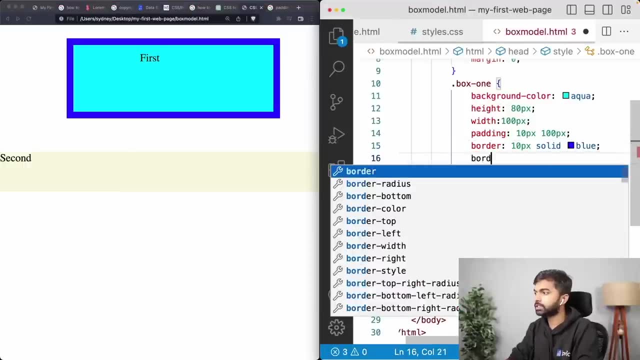 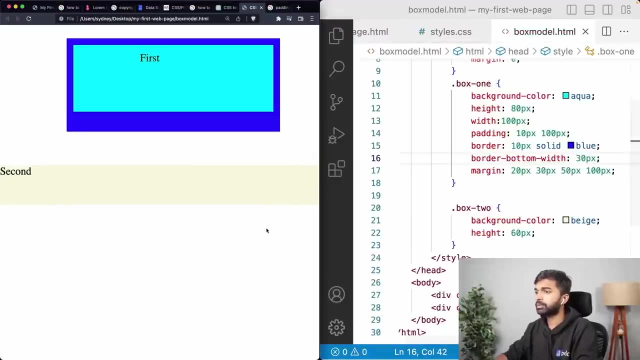 always get confused. All right, So that is margin and padding. Now here's one interesting thing I want to point out. So I hope this is all clear, And you can also, of course, go say border bottom width is 30 PX, and that is going to just change. 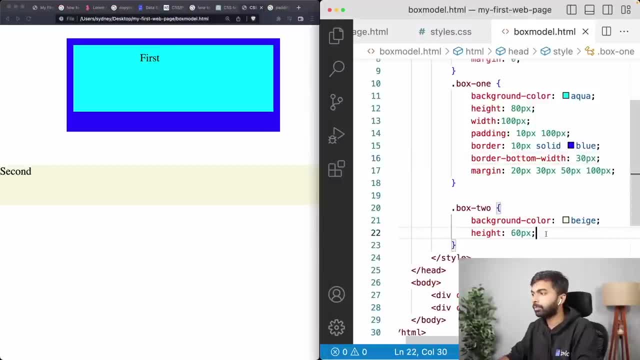 the border bottom. Wait, here's one interesting thing I want to point out. Let's say we give this a padding as well, adding 20 PX. Okay, So now it has some padding. and let's say we give it a border, border, 10 PX solid red. 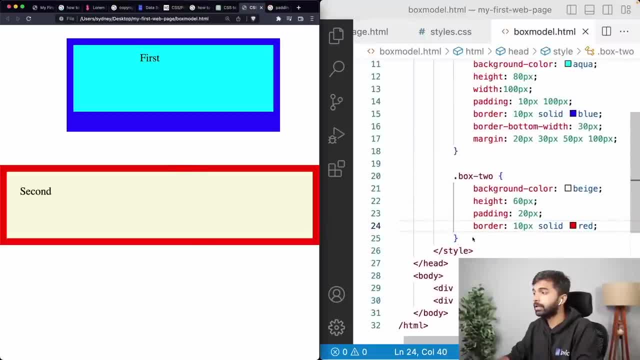 Now it has a, now it has the second box as a border As well. Now let us give it some margin, specifically, Let me give it some margin top. Okay. So notice, keep your eyes here, keep your eyes here, and I'm just going to add a margin. 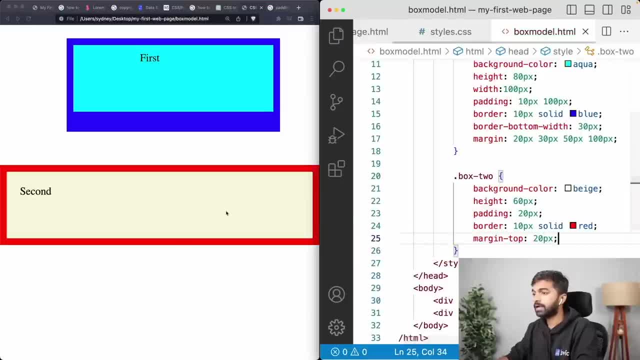 top of 20 PX and let me just save that and reload. You can see nothing happened. So what happens is that margins between consecutive elements can collapse into each other. Okay, So what happens is: this has a margin bottom of this has a margin bottom of 50 PX. 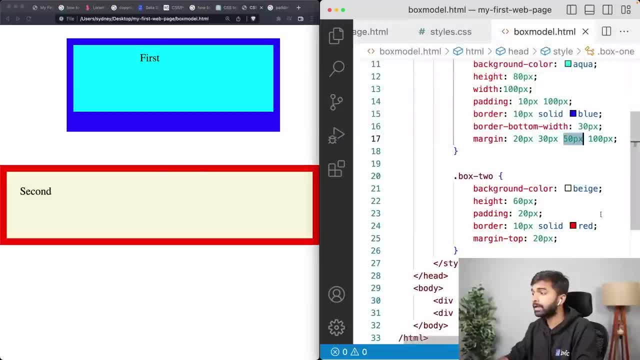 You can see here it's coming from, here It's: it has a margin bottom of 50 pixels and this has a margin top of 10 pixels. So when you have two elements side by side or one above the other and both of them have. 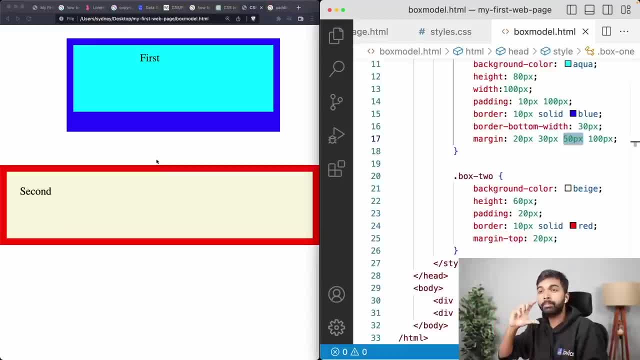 margins, then both those margins collapse into each other and only the bigger of the margins is maintained. Okay, So even if I had, let's say, margin 20 PX all around and reload this page, you can see that a margin got added here, a margin got added here, a margin got added here, but a margin. 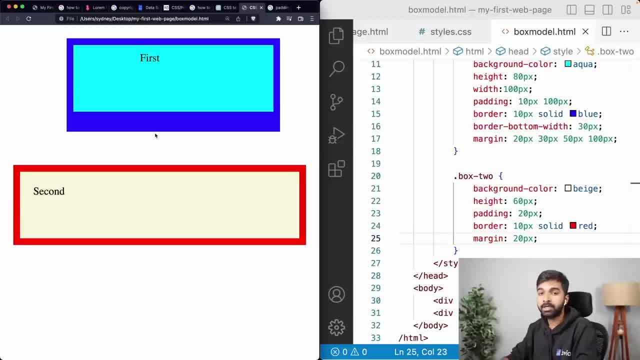 did not get added here, because this margin is shared with the margin of the above element. Okay, So you should keep in mind that margins of successive elements collapse. Don't worry If you forget this, you're going to figure it out when you build your web pages. 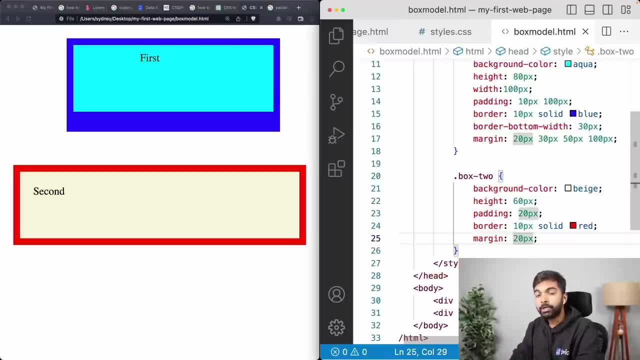 Anyway, here's another thing that I want to tell you. you can use another margin setting called auto. So let's say I said margin top to be 20 pixels, margin uh, right to be auto, margin bottom to be 30 pixels and margin left to be auto. 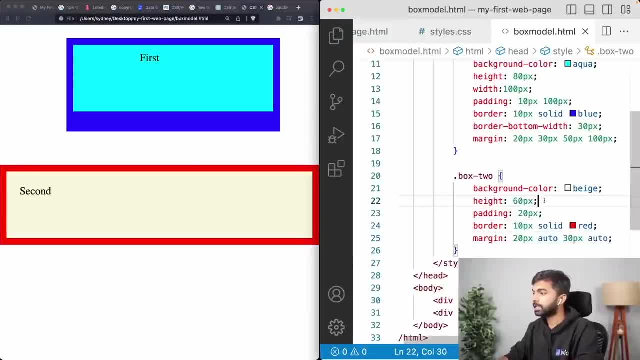 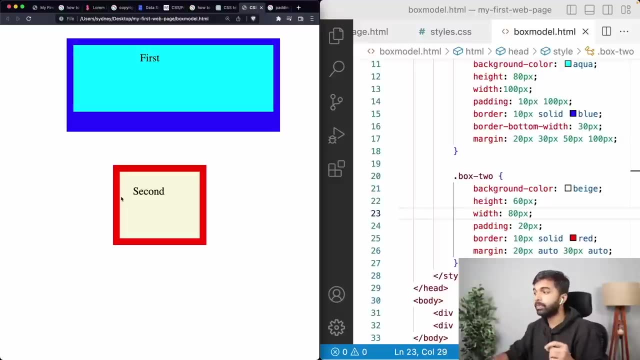 What happens is- and I also said a bit for this- Let me set the width to 80 PX. You can see what happened: that the width constraint how much space the div can take up. because you've set a width properly And then the margin on the top and bottom apply as usual, but because we've set the 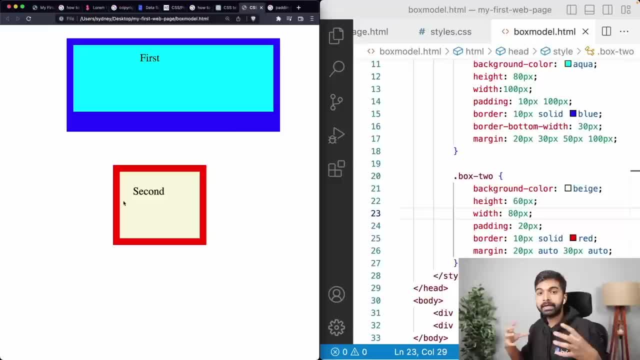 margin left and right to auto. both of those are automatically adjusted to be equal, And this is a very powerful thing. This doesn't work with top and bottom. This works with left and right only if you set the left and right margin to auto. what 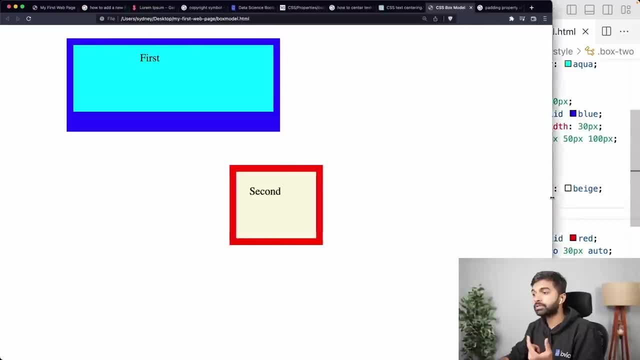 that does is that It centers the div horizontally on the page. You can see as I change the size of the browser, the second div stays in the center. So that's a good, neat trick to center a div horizontally on a page. 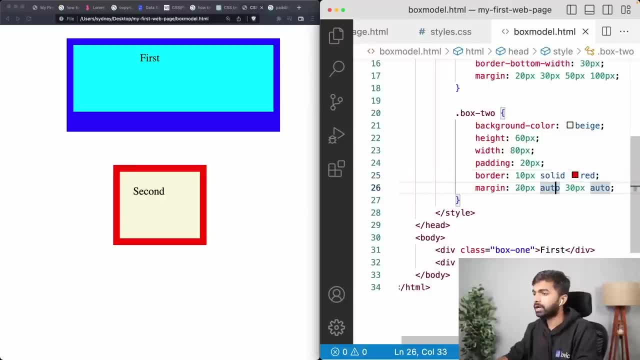 Just set the margin to auto for left and right, All right. So that's about the CSS box model And, generally speaking, if you want to, if you have a doubt about where a particular space or margin or padding is coming from, here's what you can do. 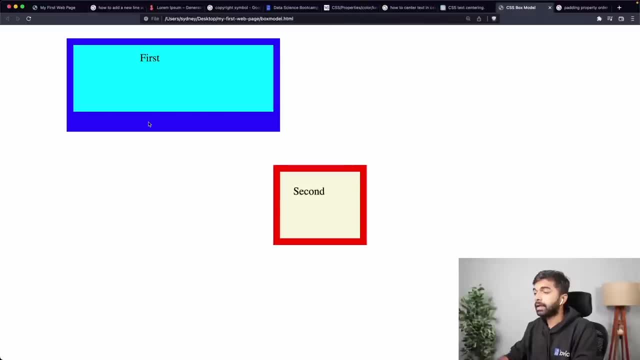 Let me just zoom, Let me just make this full screen, Let me just make this full screen for once. And you can right click on an element- and this works in Chrome or brave browser- doesn't work in Safari, I believe- but right click on an element and click inspect. 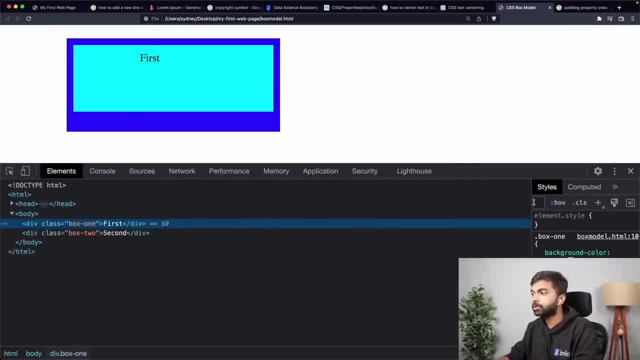 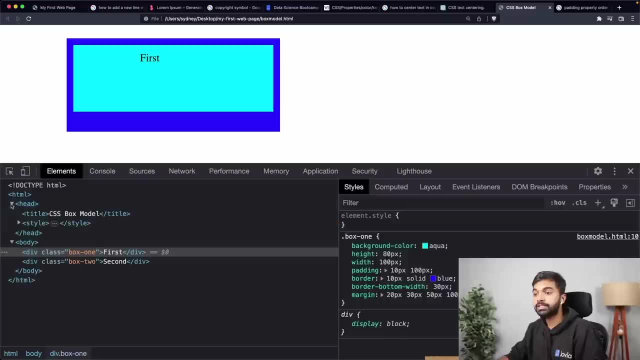 And when you click inspect, the browser is going to show you the actual HTML structure of the page. So you can go into any webpage on the internet, You can right click and you can inspect and you can study the HTML source code of the page. 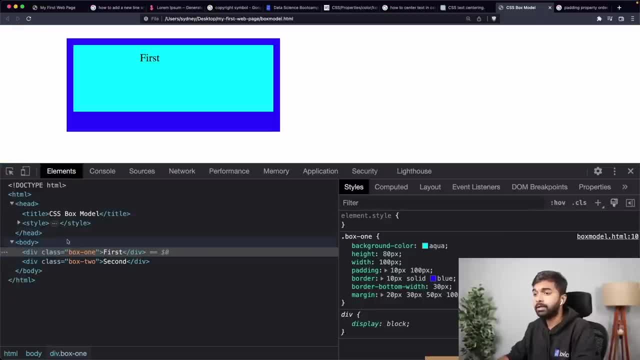 You can see here, it has all the entire style. It has the entire body div, all of that, And when you hover over a particular div, It shows you what that div looks like, And specifically the green area, the green area that you're seeing. that is the content. 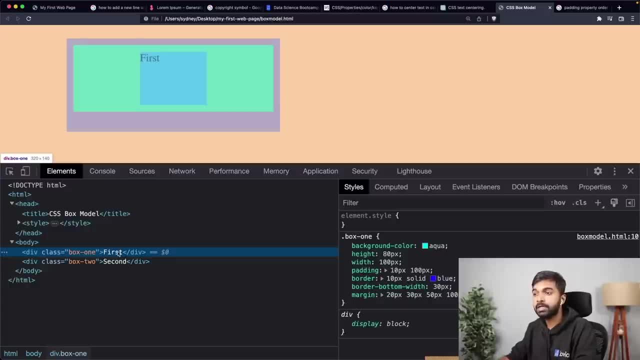 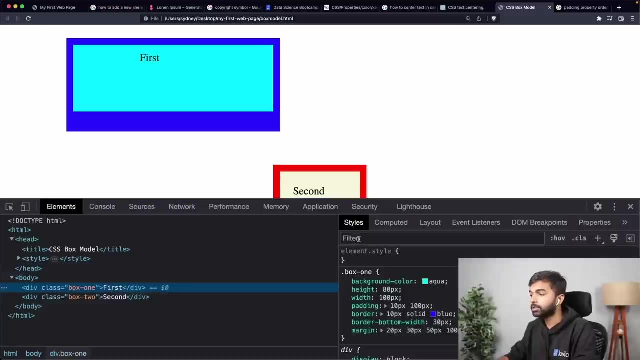 of the div, including the padding, And then the orange area that you're seeing. that is the generally the margin of the div. Okay, You can see the orange area is the margin and the green area is the content. You can also come in here on the right and you can study all the styles that are applying. 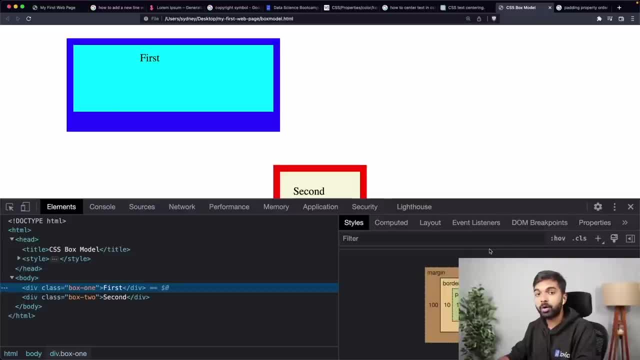 to this particular component And you can actually look at the box model for that particular. So if you select box one, You can see it's box model here. You can see that it has the size hundred by 80 and it is highlighted and it has a padding. 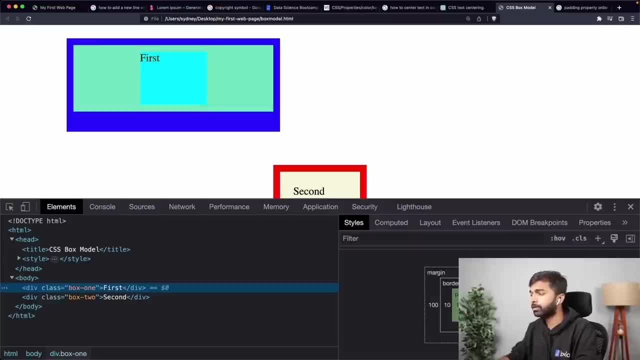 of 10 at the top, a hundred at the right and then 10 at the bottom and a hundred on the left, And you can see it has a border of 10 on each side. And finally it has these margins: 20,, 30,, 50 and a hundred on each side. 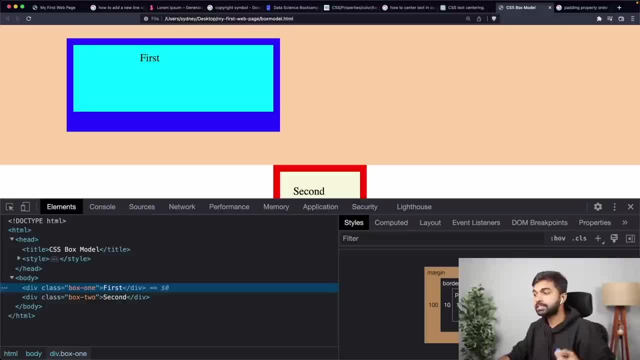 Okay, So that is one great way for you to explore the CSS properties. If you scroll up, you can also see what are all the CSS properties that are applied here. You can actually turn off these CSS properties or you can add additional CSS properties. 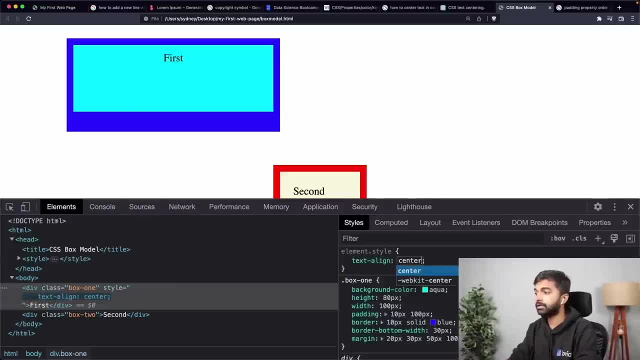 For example, you can say text align center and that is going to apply that additional CSS property. So this is a great way to just experiment with your webpage in the browser itself before you go back and make some change in your code. Okay, 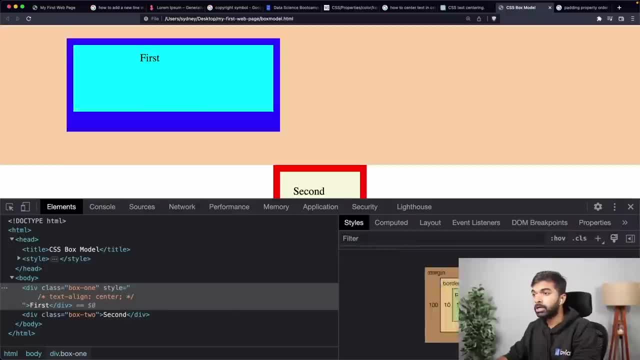 And if you reload the page, all of these changes will go away. but the box model is useful to explore, Then the CSS properties are useful to explore and you can also add additional properties or you can change the values of specific properties. Let's say, instead of aqua, I want to change this to gold. 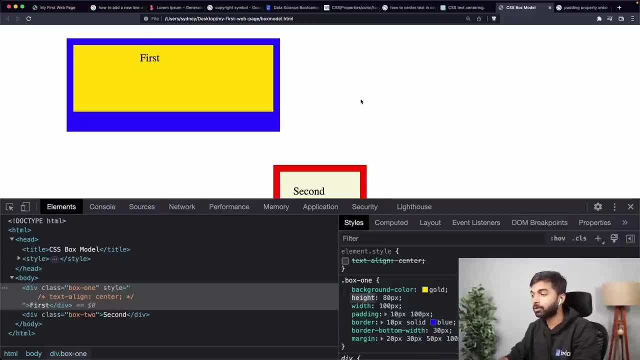 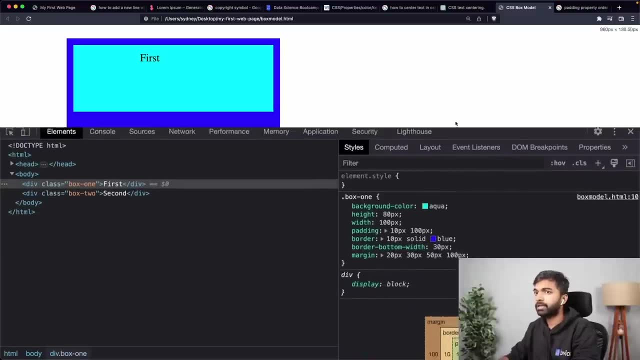 I can do that here as well. And again, all of this is just changing in the browser. it's not going to go and save anything, All right, So that's an interesting way for you to explore web pages either, if you're not able to see. 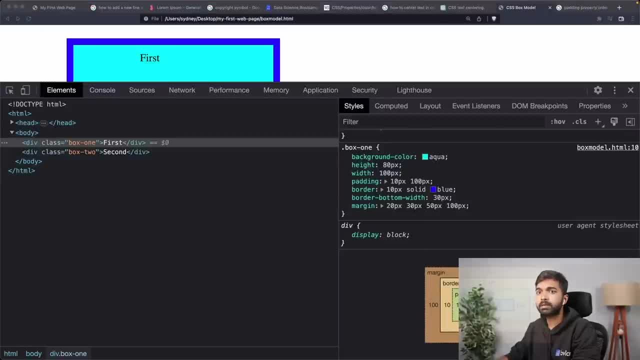 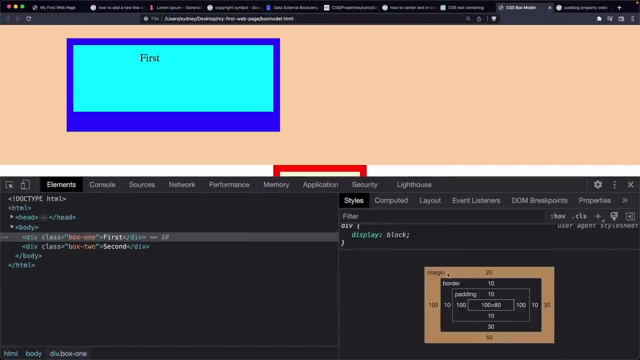 the box model. let me just turn this off here. Yeah, So this is the box model. You can see that if you scroll up, you can see here that you have the box model. you can see the margin, you can see the border, you can see the padding and you can see the. 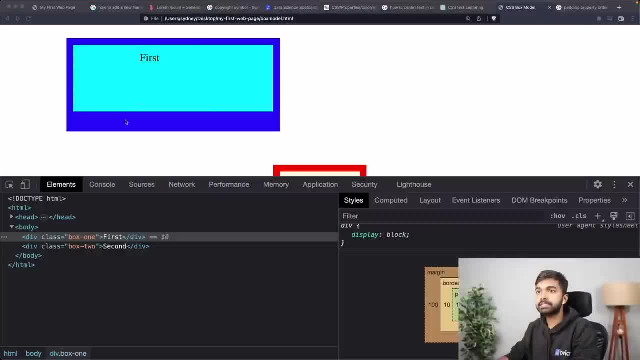 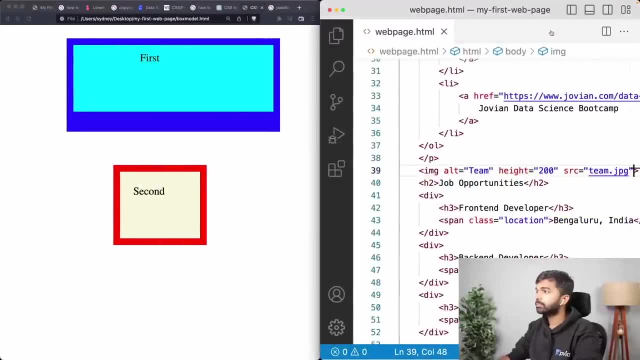 size of the box itself. Okay, That is the CSS box model. Okay, So let's go back into the page webpagehtml, and let's also open up stylescss. So let's go back to stylescss. By the way, you can use command P within VS code to open stylescss. VS code is really. 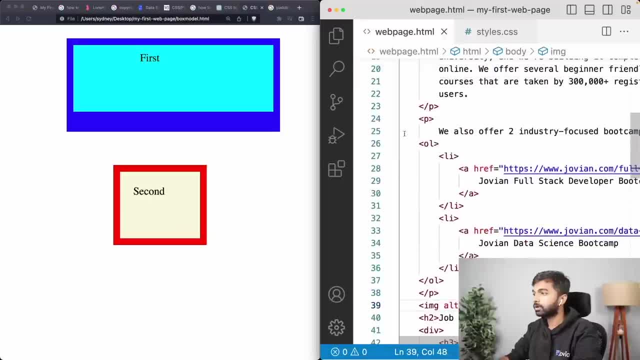 nice for coding. It makes the job really, really easy. You can also close or collapse some of these HTML tags in case you don't want to see them, And that way you can reduce the structure of your page. So I'm just opening everything for now. 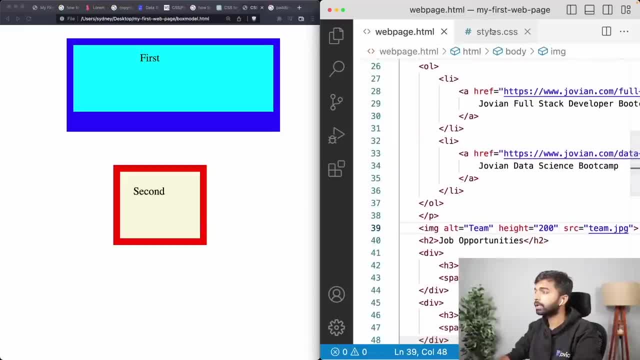 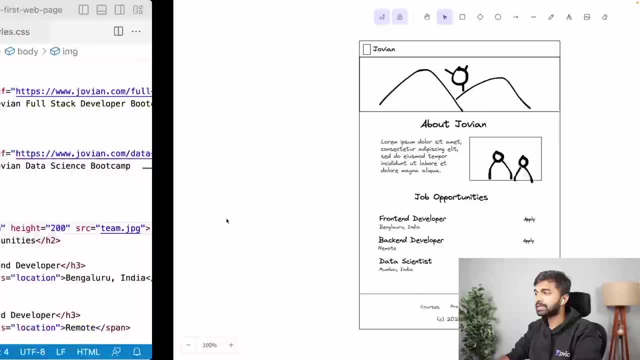 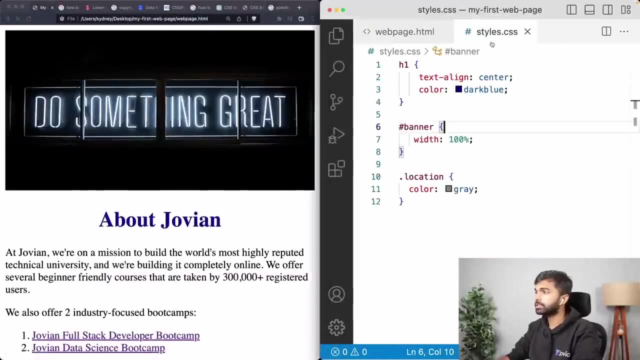 But you can do that. You can do that if you want. Okay, Then let's go back here to my first webpage, And let us now try and achieve this layout step by step. Okay, So the first thing I'm going to do is go into stylescss, right at the very top. 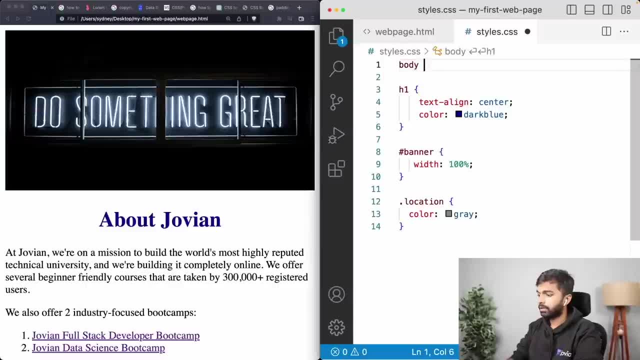 I'm going to go into body And I'm going to set a few things right, Because every browser has its own setup of the body, Although its own margin and padding. you can see here that there is some white space around this image, even though I've set its width to 100%. 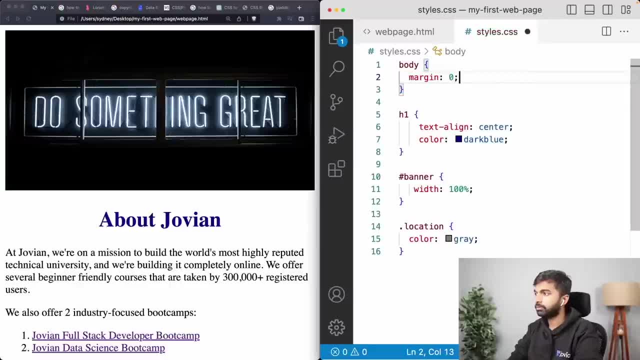 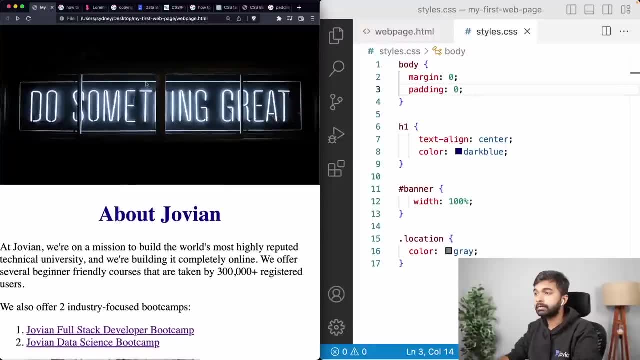 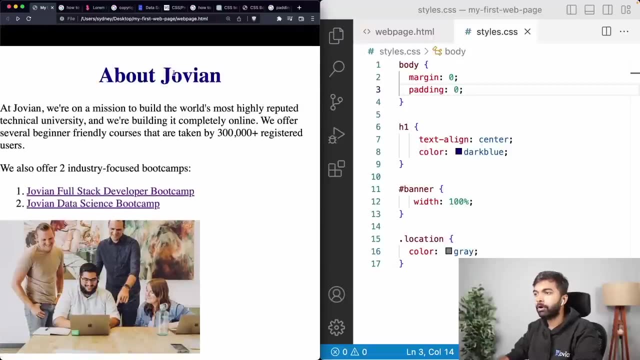 So, within the body, I'm just going to set margin as zero and I'm going to set padding as zero as well. Great. So now this is completely out there touching the edges, Okay. One other thing that I want to do in the body is I don't like this font, which has these: 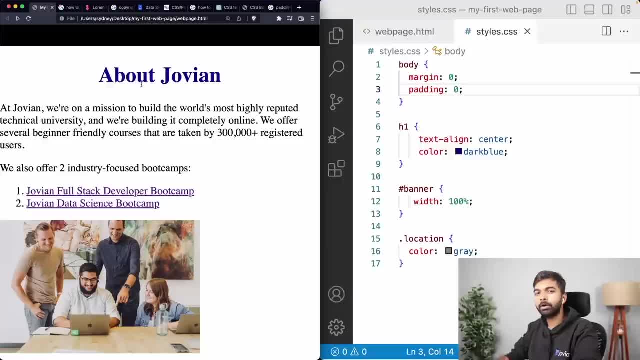 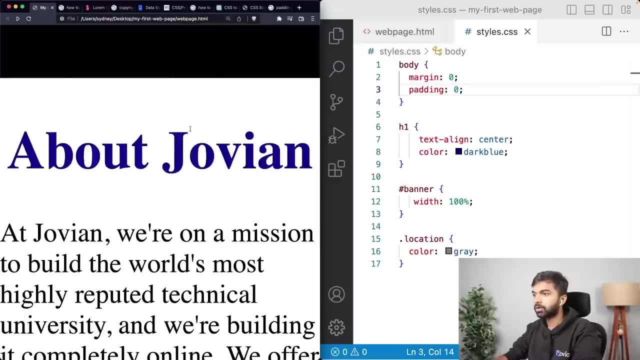 things sticking out of the J. You can see right at the top. It has this old look. Okay, This is called a serif font, This small piece sticking out of the J, This thing over here is called a serif And similarly, this is called a serif. 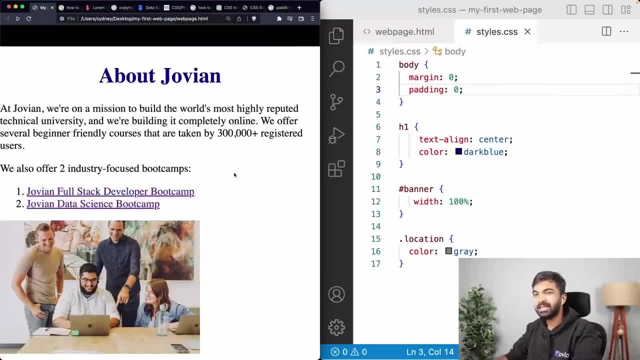 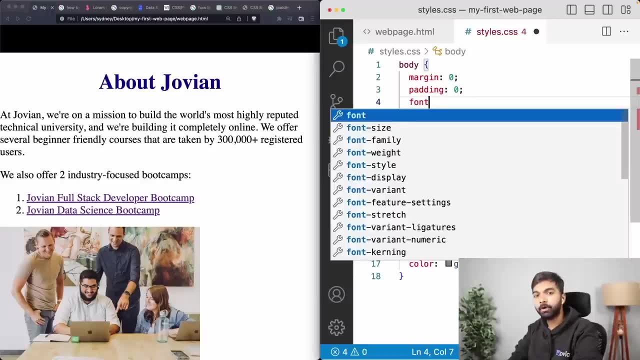 This is what is called a serif font. Generally speaking, most modern websites are built using sans serif fonts, So I'm just going to go in and change the font Now. the way you set the font is by setting the font family, And there are many font families that are available on the internet. 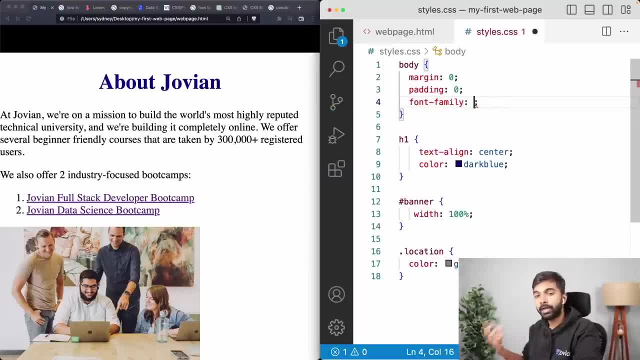 By default, browsers support several font families And your operating system may have certain font families, and then you can include new font families from the internet, from a resource like Google fonts, and we'll do all of those things, But for now I'm just going to say sans serif: 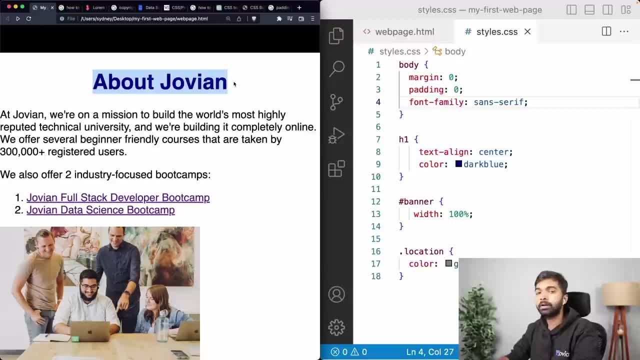 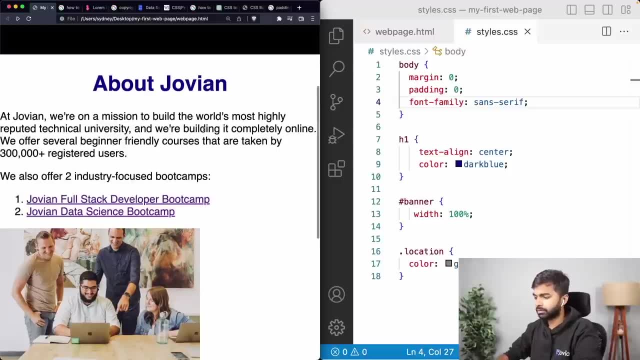 Okay, What that does is, if I reload the page, you can see that now it looks a lot more modern. Now it doesn't have those things sticking out of the J and out of the B and all. So that's one other thing that we have done. 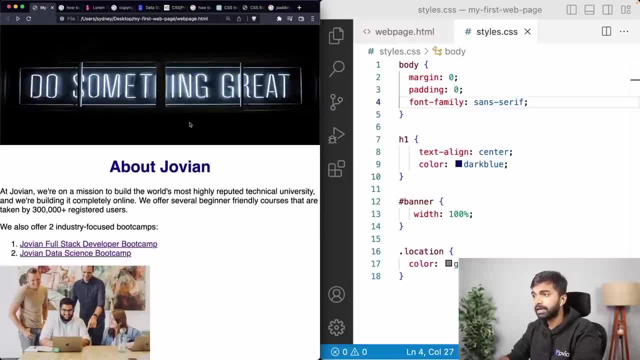 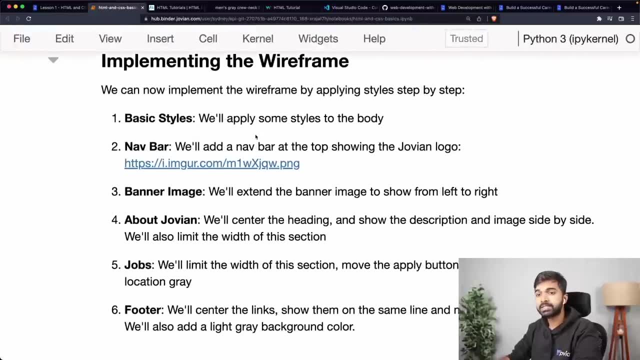 Let me just zoom out a little bit, Okay. So now we've done that, Let's start fixing. So let's start implementing the wireframe by applying the styles step by step. Okay, So the first thing that I'm going to do is I'm going to add a header. I'm going to go. 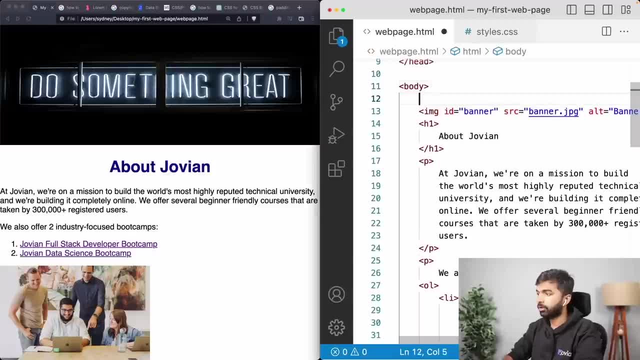 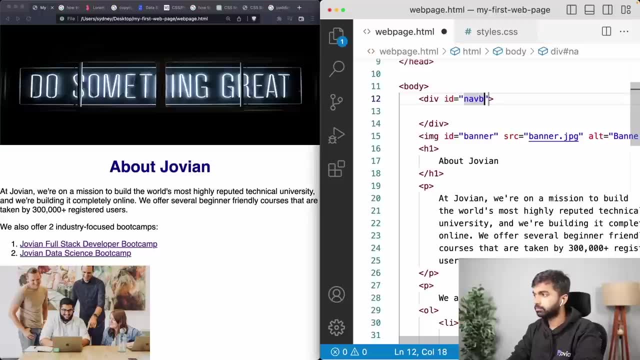 in into web page or HTML, And here, right at the top, I'm going to create a div And I'm going to give it the ID navbar. Okay, this is going to be the navbar right at the top. So over here and inside this, I'm going to need an image. I'm going to put that image. 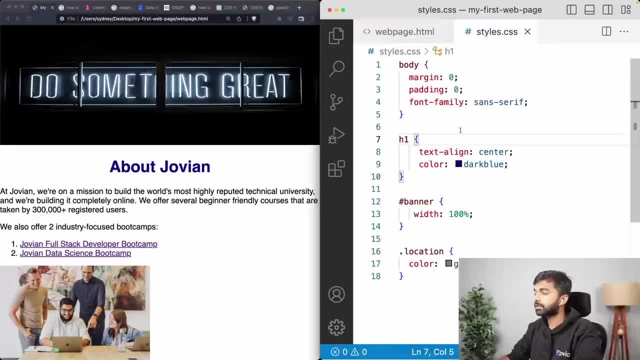 in in just a second. But let us give me, let us give some styles to the navbar. Let's go in here, let's add- I've given it the ID navbar so I can select it using hash, And let me then set the height, or let me just give some padding to the navbar. 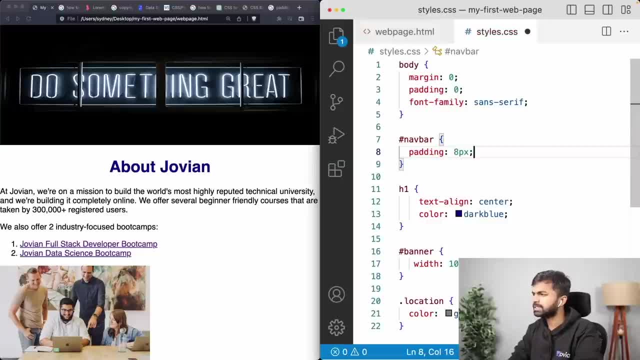 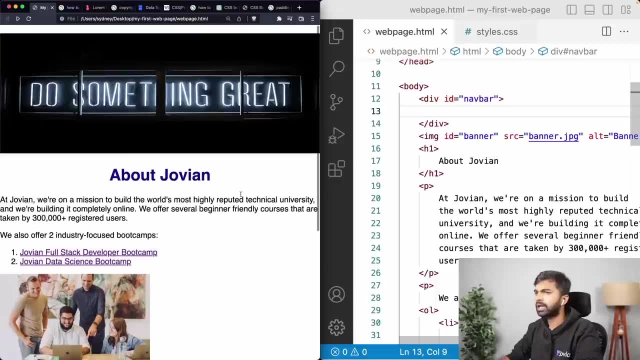 Let me give it a padding of eight pixels. let's just set it to eight pixels for now. Okay, nothing happened. Oh, there it is. Yeah, So that is our navbar, right there. It has eight pixels of padding. that is why it just showing up like that. 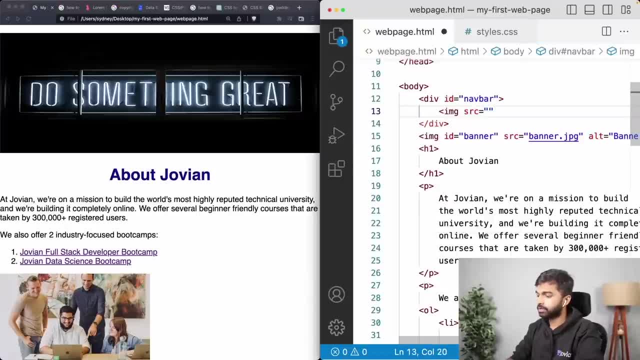 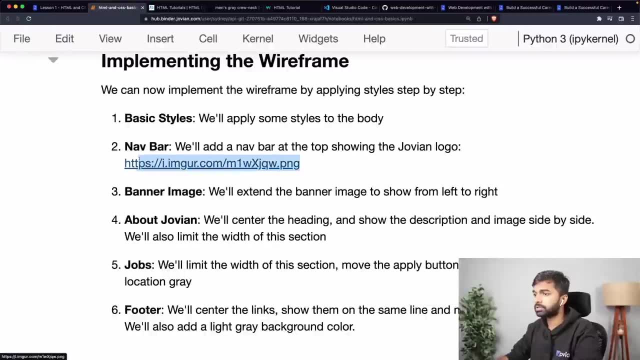 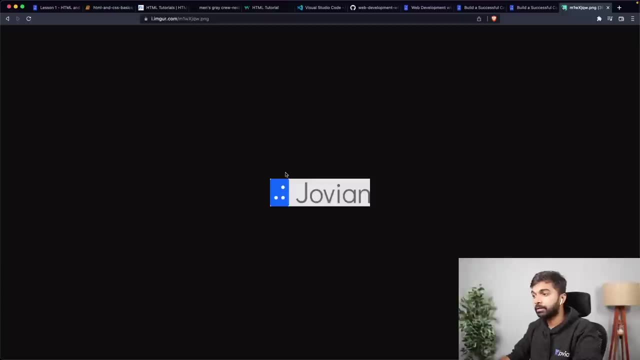 Let's now put an image under it. So image SRC- what is going to be the location of the image? Well, I have picked out a Jovian image logo here, So I have this image posted online. Okay, so whenever you're using an image from the internet, make sure that you're actually. 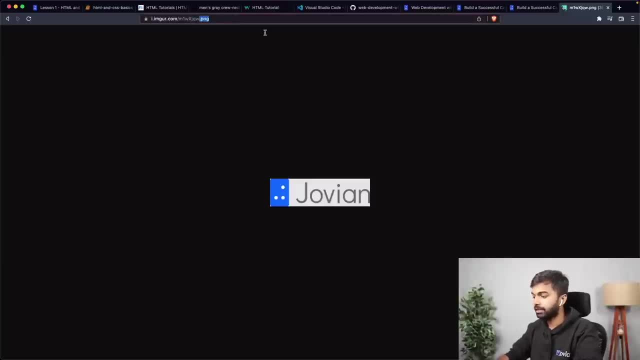 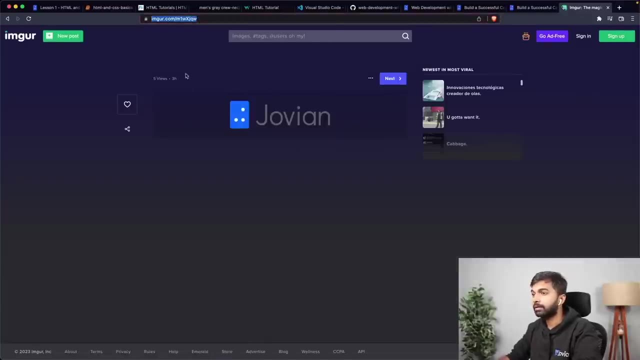 getting the link to the image itself and not the link to a page containing the image, for example. So let's say I have a page that contains the image, But I shouldn't put this in the SRC, because then the browser is going to try to fetch. 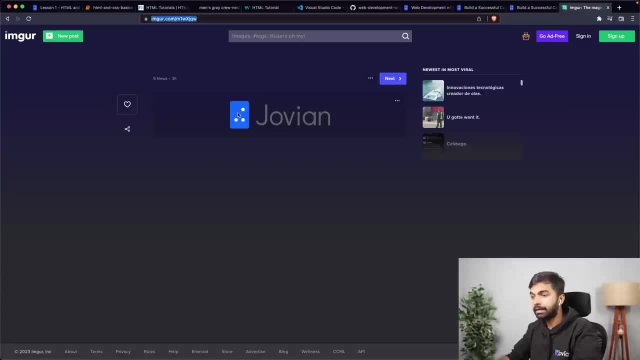 this entire page as an image. No, So you can do two things: right click if you want to include an image from the internet on your web page. right click and say copy image address And then just put that here in SRC. Or you can right click and say open image in new tab and then grab the URL of just that. 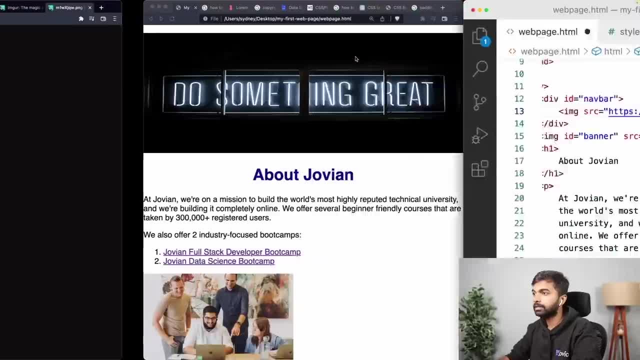 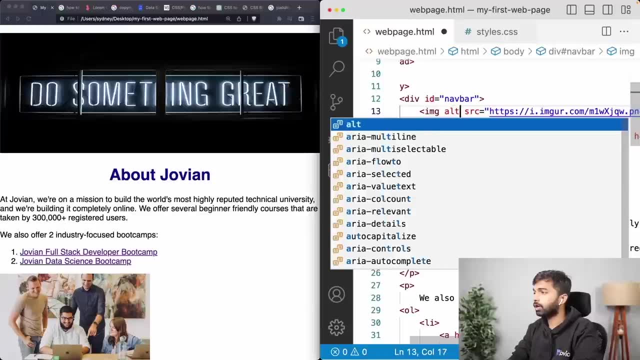 image. Okay, So I'm going to put in a new tab and then grab the URL. that is the safest way to do it. Alright, so IMG SRC equals that, And I'm just going to give it an alt because that's a good practice. 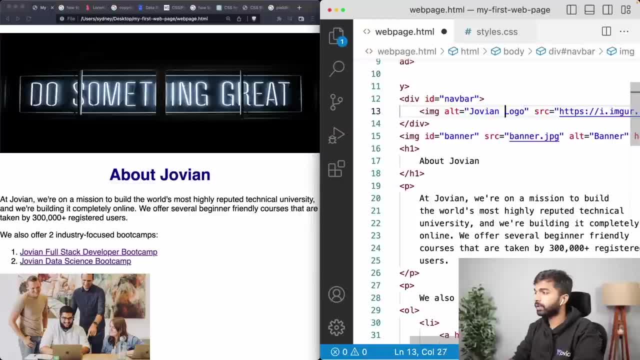 So I'm just going to say Jovian logo and I'm going to give it ID logo, All right. And now this image should show up here, but it's obviously too big. Let's go in here and let us set the. we have the logo, which is an image. 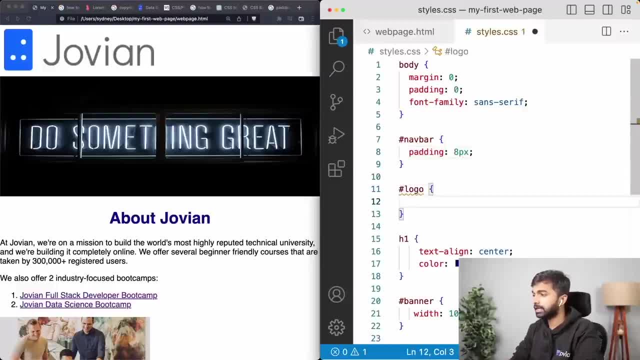 All right, And now this image should show up here, but it's obviously too big. Let's go in here and let us set the. we have the logo, which is an image. Let us set its height to 32px. Okay, that looks nice. maybe even 30px. 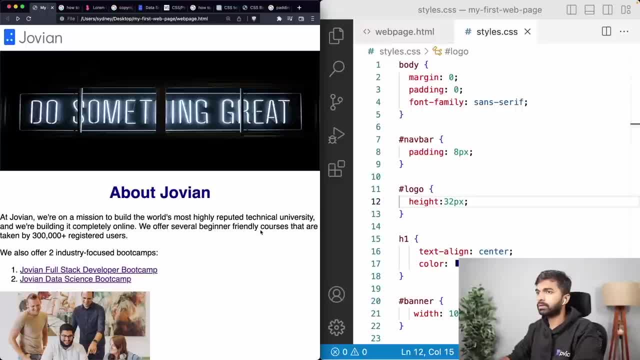 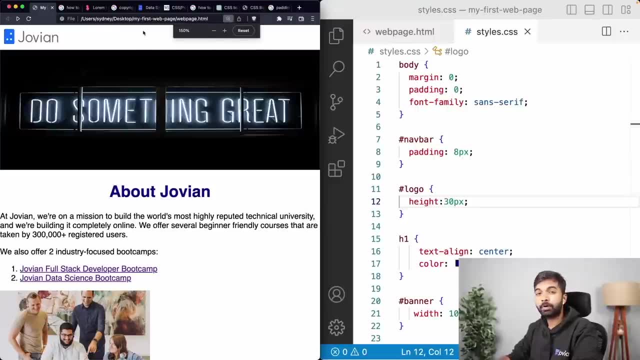 And remember this is zoomed in. I've actually zoomed it to about 150% In your, on your side, it may actually look a little smaller Alright, so that is starting to look good. Is there a margin for the snap bar? 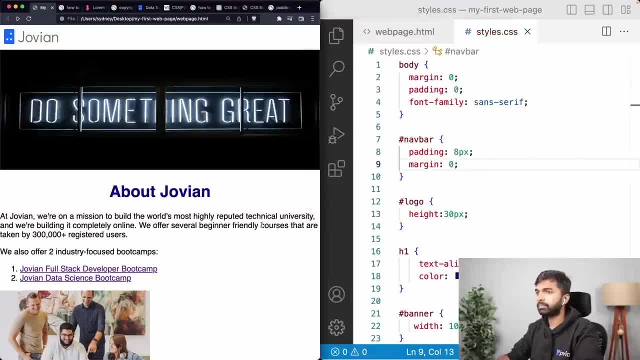 Let's set the margin to zero. Let's make sure that there is no margin here. Okay, there's no margin, Okay, There's no margin, And this is looking good. So now we have this. nice, it's looking a bit unequal. 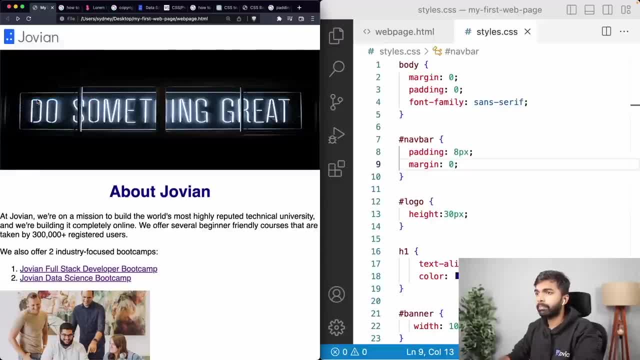 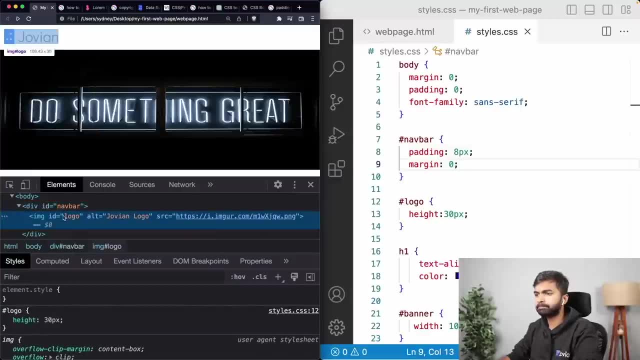 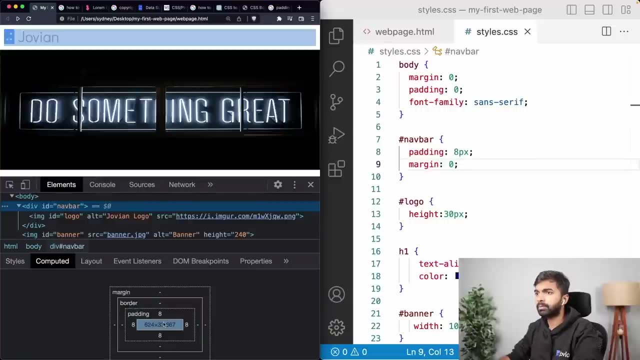 You can see on the top and at the bottom we have unequal space. So we can verify why there is this unequal space by checking the navbar And looks like. well, looks fine to me. Okay, I have no idea why this is unequal. 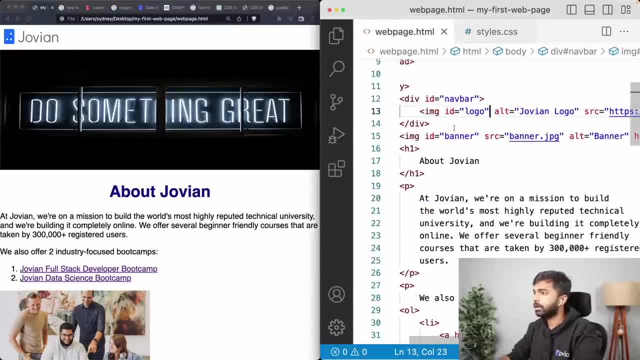 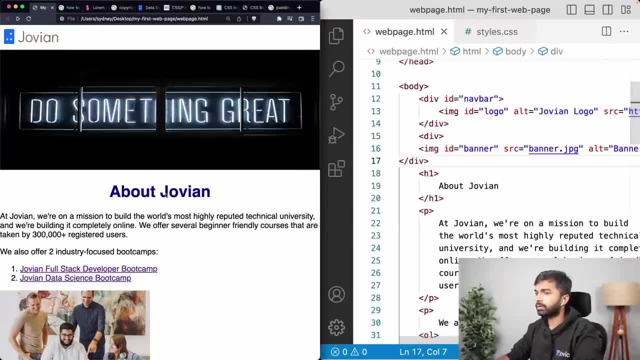 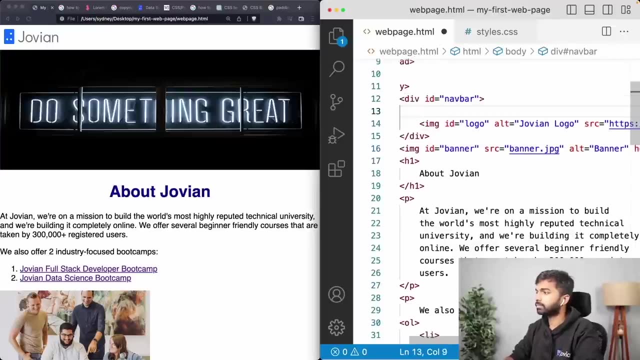 That is something in CSS. Sometimes you have to Figure out ways to fix, But in any case, I think one. one way we could do this is maybe just chuck this into a div. No, that doesn't do it. Oh, that's the wrong thing. 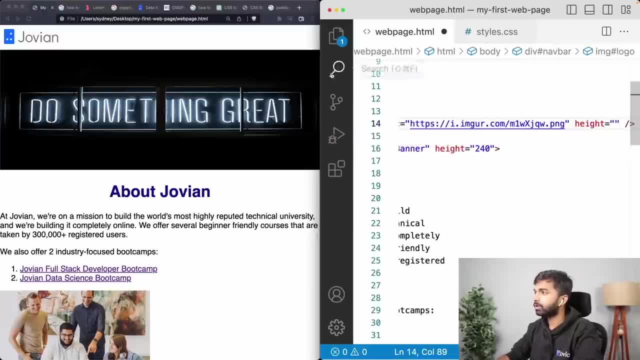 Maybe I can just set the height directly here. So height equals what is the height we need for the image: 30px. So let me just set the height to 30 here directly. Sometimes that tends to do the trick And let me remove that. 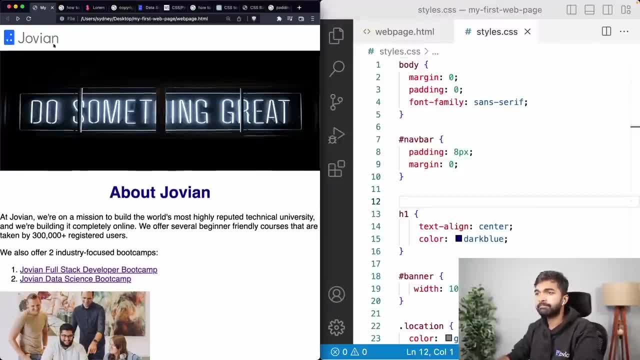 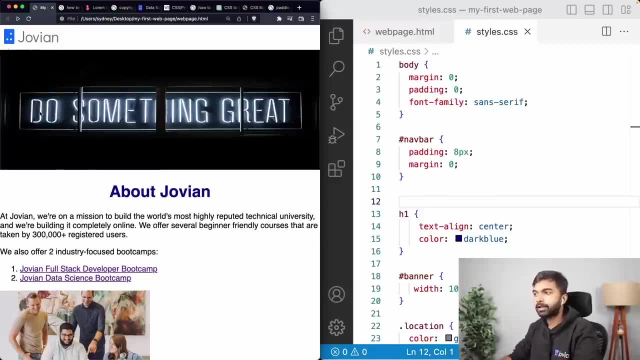 Remove the height from here. I've just set the height directly. okay, still doesn't do it. So you're going to run into these issues in CSS where something is slightly off, And I normally just keep these towards the end so that I don't worry about them immediately. 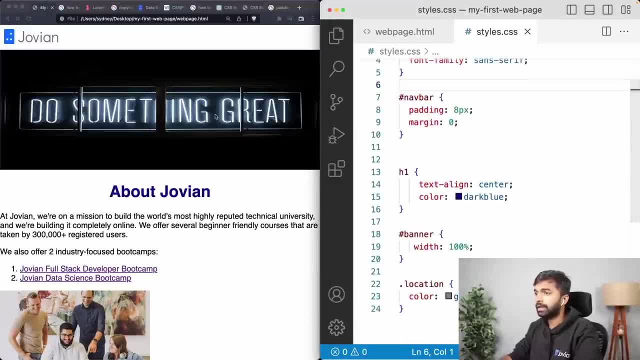 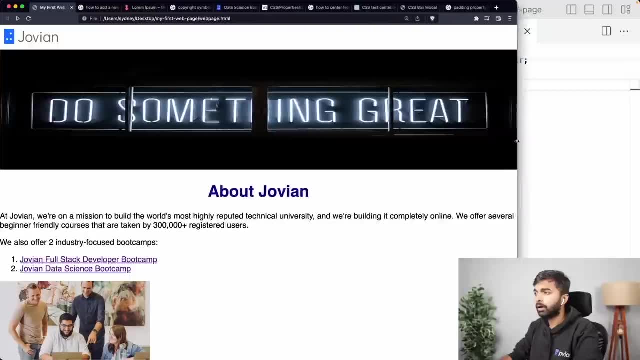 But, in any case, now we have the navbar in order, And then let us fix this image. So this image looks fine, But the only trouble here is that the image is stretching. Okay, Now, what I want you to do, what I want this image to do instead, is just to cover the entire. 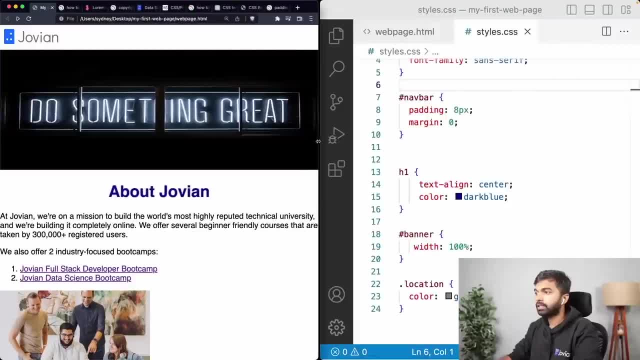 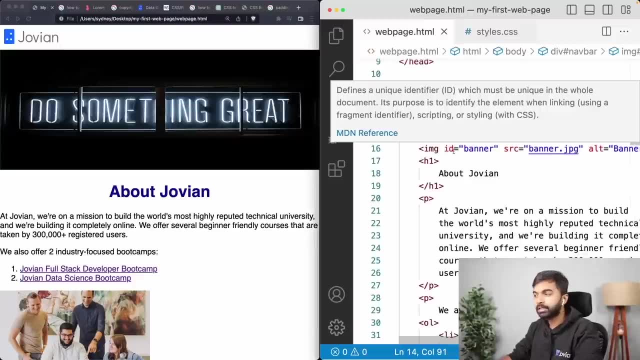 area that is available to this image Instead of stretching, and the way you can do that is by adding something called an object fit into the image. Okay, again, something that you can look up. So this image has the ID banner. I'm going to come in here and I'm going to add for 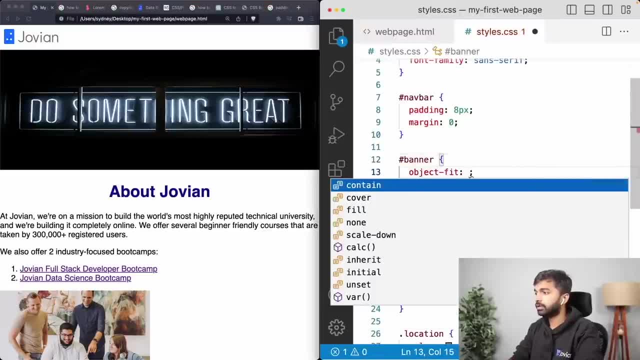 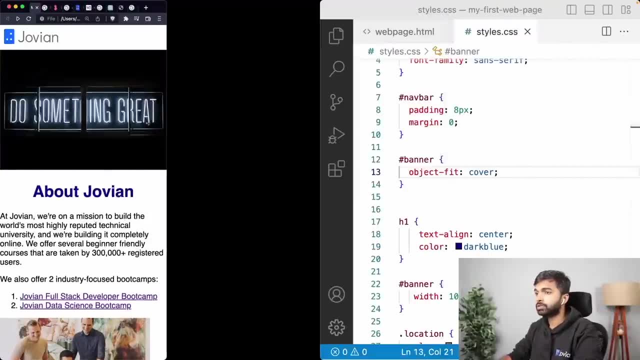 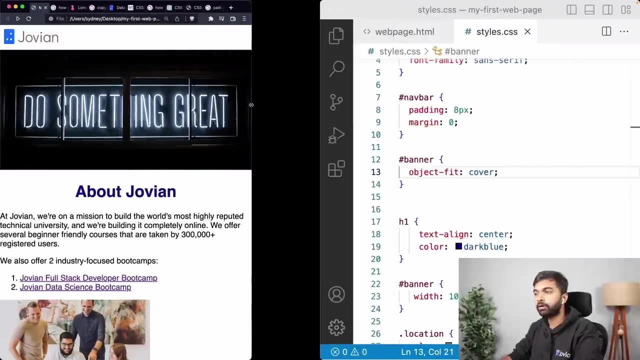 banner. I'm going to set object fit power, okay. And now you can see that whether I zoom it in, or whether I increase or decrease the size of the web page, the aspect ratio of the image isn't changing. So this is the way you you fix your stretchy images. you simply set object fit cover whenever. 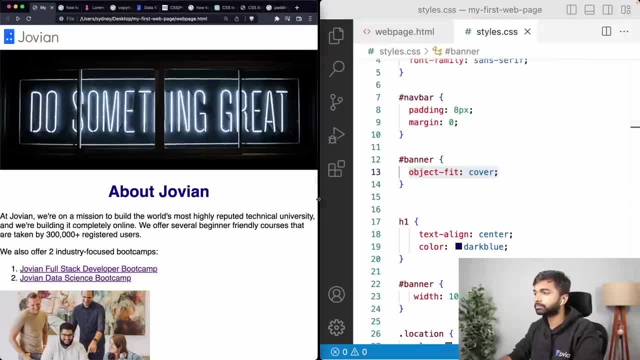 you see that an image is stretching. Okay, So that takes care of our navbar, that takes care of our banner. Fine, Let's fix the about Jovian, I think we don't need the dark blue color. I'm actually okay with the black color. 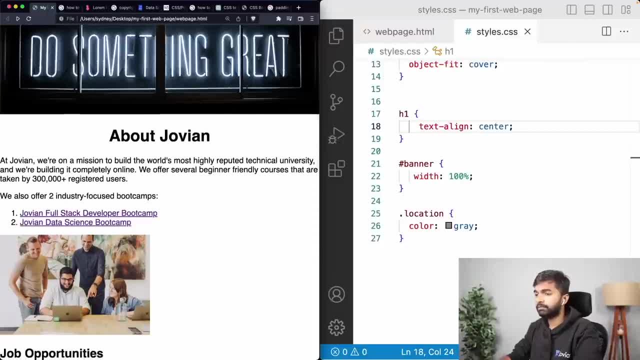 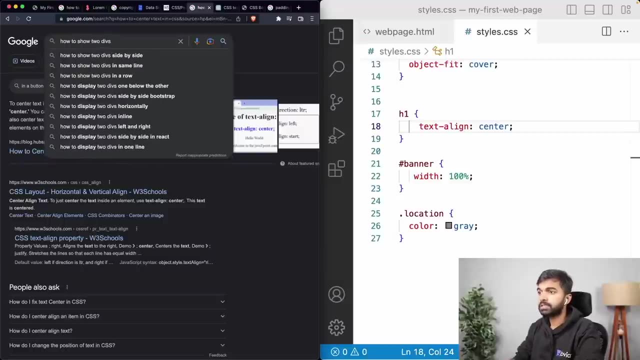 And now, here we have these two things. So we have the left and we have the right. we want to show two divs side by side, Each taking half the screen, And again, this is something that I would search online. I would say how to do two divs. 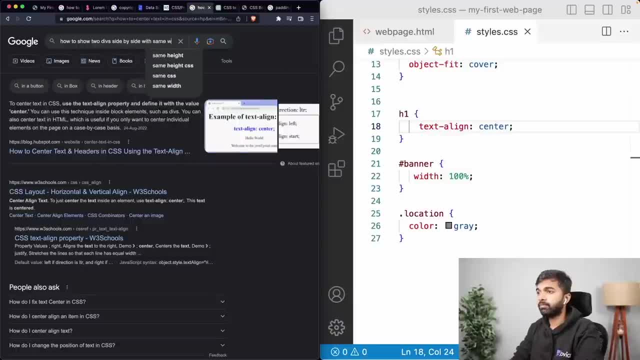 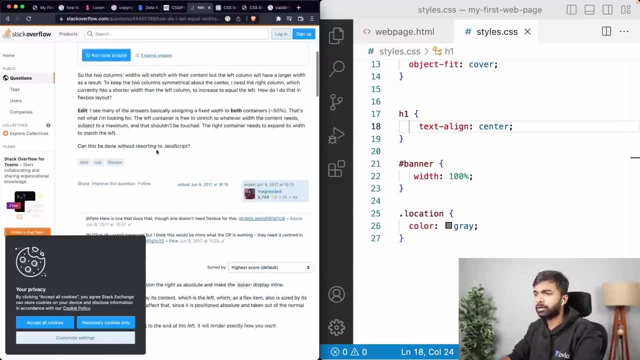 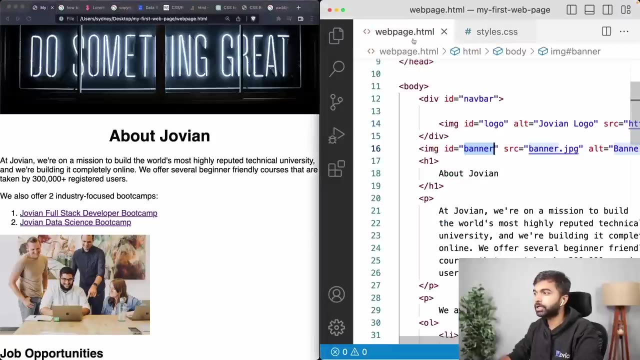 side by side with same width, And you can see I've searched this already. I think this one was one that I found useful. So, yeah, you can explore this a little bit, but I'm just going to go ahead and show you the solution here. 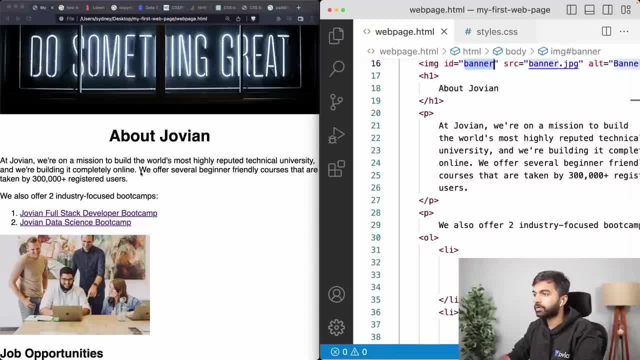 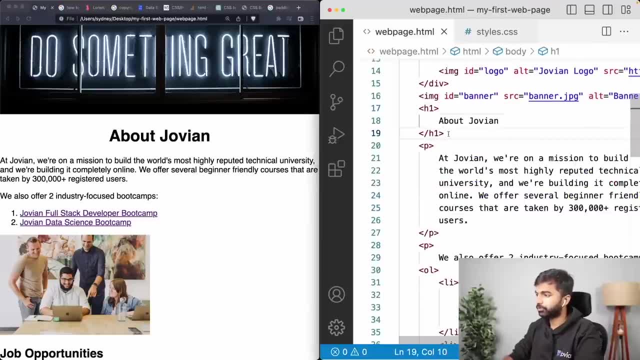 Whenever you need to show, Show two divs side by side. what you need to do is first make sure that this content and this content both are within a div. Let's take a, let's see, let's go to about Jovian. 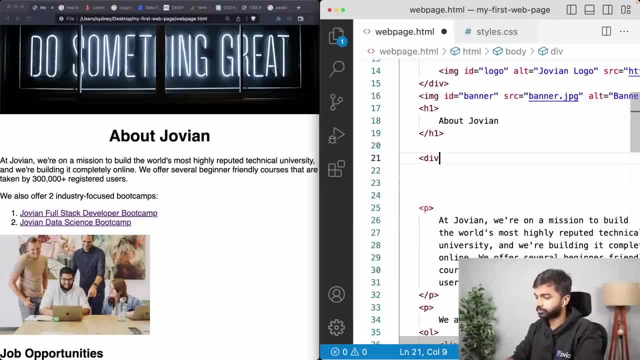 And under about Jovian. first let's create a div called description. Let's give it the ID. Let's give it the ID about: okay, this div is going to capture everything under the about section. And then let's create two divs inside it. 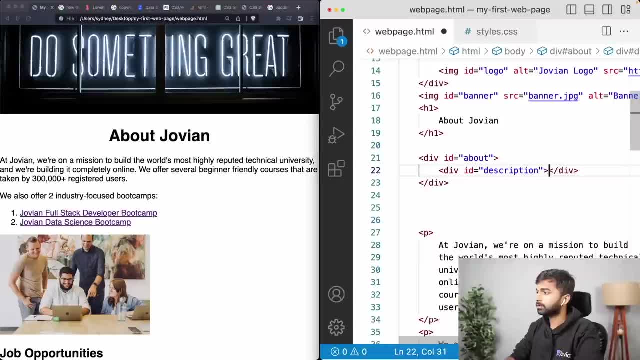 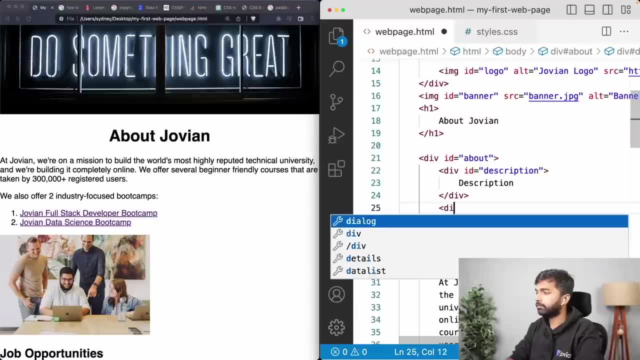 Let's give this the ID Description, And this is going to be the description. And then let's create another div. Let's give this div the ID team, And this is going to be the team image. Okay, so we have created two divs. 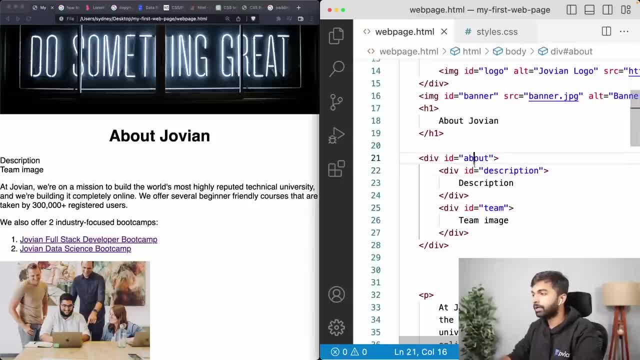 One is called description and one is called team. Now, by default, divs are going to show up one below the other in HTML. If you want to change that, here is a quick trick you can apply If you want the divs inside a particular outer div to flow not horizontally but vertically. 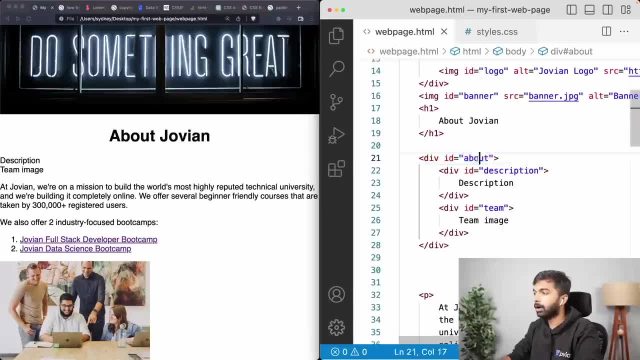 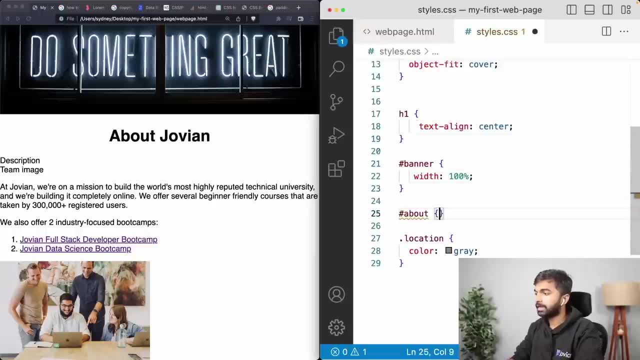 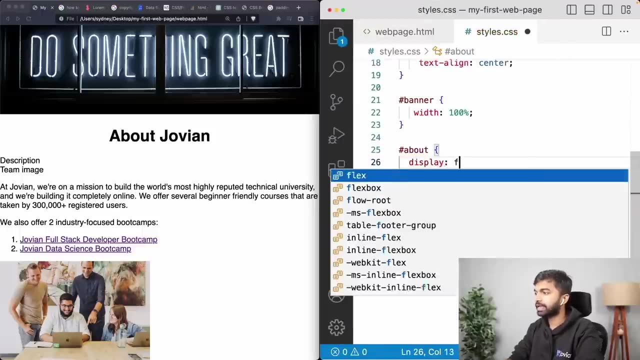 And what you can do is go in and this outer div is called about. So I'm going to just go into about. So I'm selecting the outer div with the ID about and I'm going to just set display flex. Okay, we're going to learn about flex. 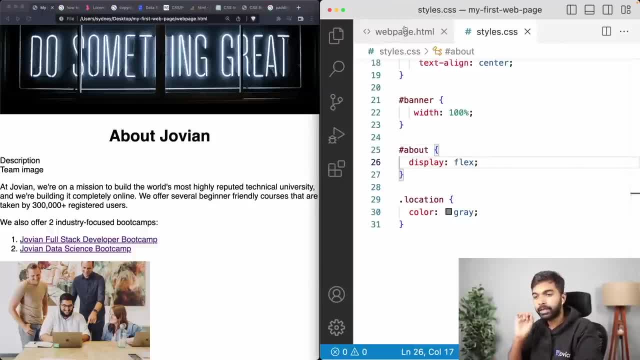 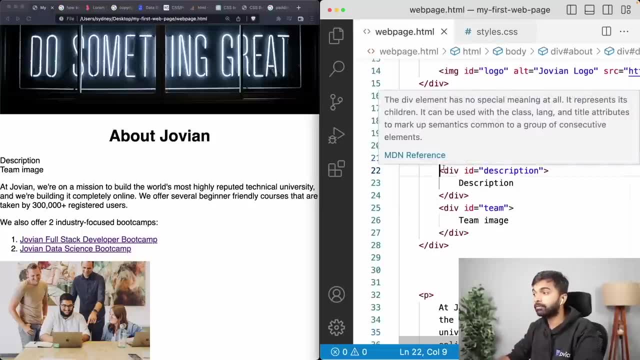 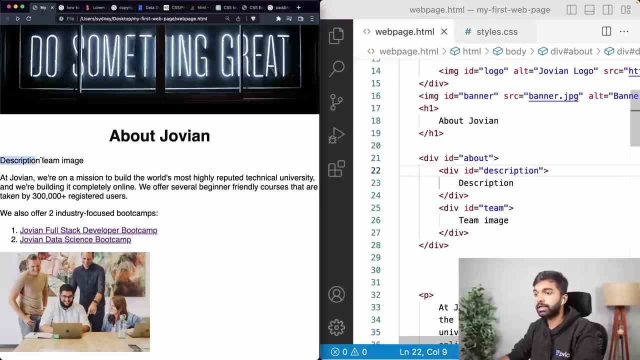 The flex display In a lot of detail later on, but the quickest or the easiest reason to use flex is to change the orientation of the divs inside an outer div from horizontal, from vertical to horizontal. Okay, and I reload that and you can see. now we have description and team image coming. 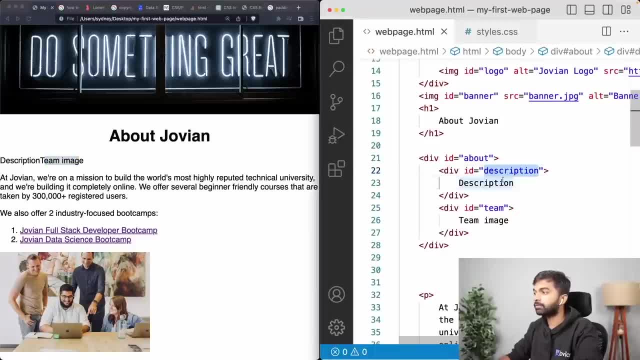 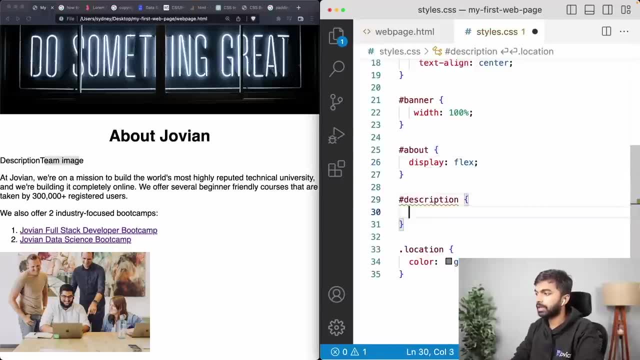 side by side. Now here's what I can do. I can set the width for description and team. Okay. so I can do something like this: We have description And I can set width 50%. what I wanted to do is occupy 50% of the area of the parent div. 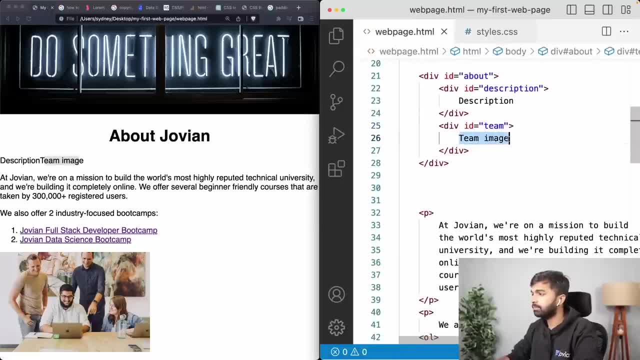 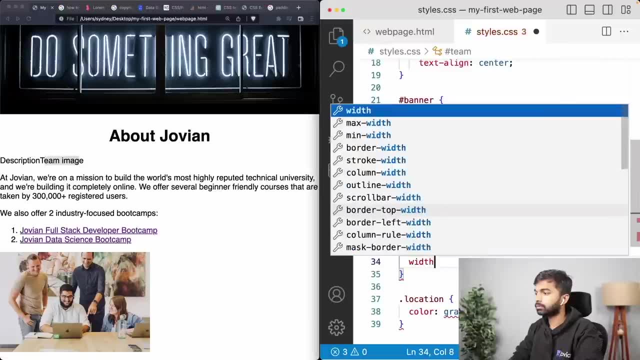 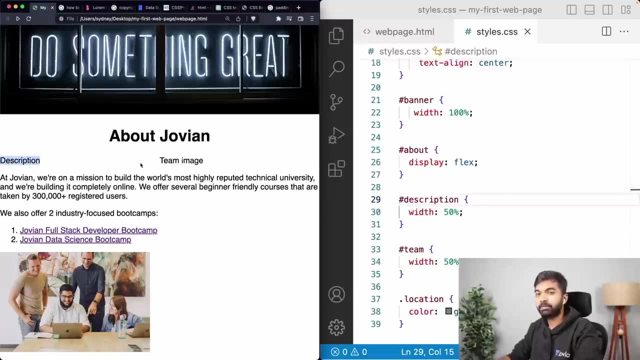 And similarly, we have this team image or this team div, and I want that to occupy 50% as well. Okay, and now you can see that description takes up 50%. If I added a background to it, you will be able to see. let me add a background just to. 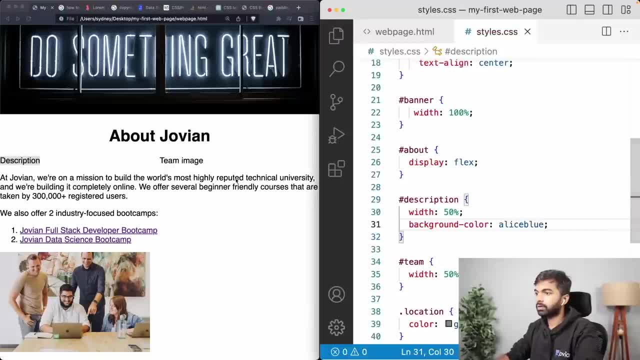 show you. Yeah, so you can see around. description there is this background of description takes up 50% and the team image takes up 50% and of course now I can go in and I can put these two pieces of content inside those divs. 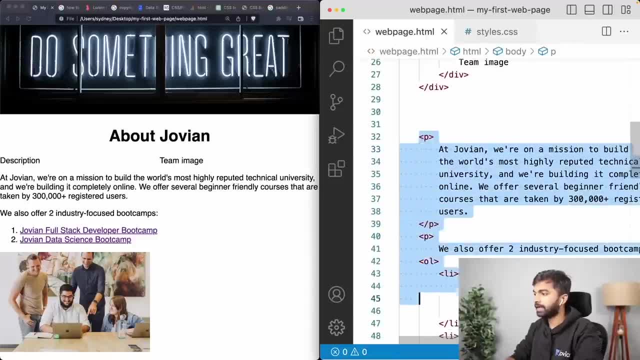 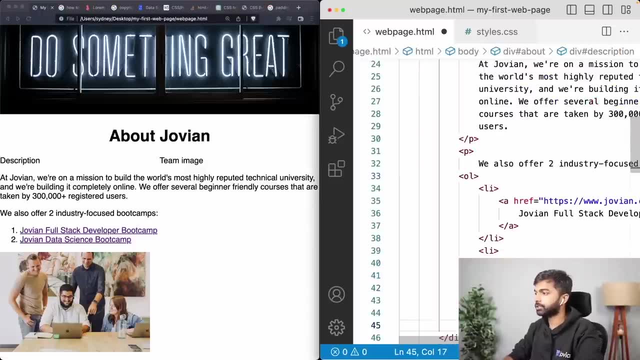 Okay, so I have this P tag with a, with this ol and all of that. So let me just grab that P tag and cut that and put this in the place of description. Okay, And let me just right click here and indent: I think it should. 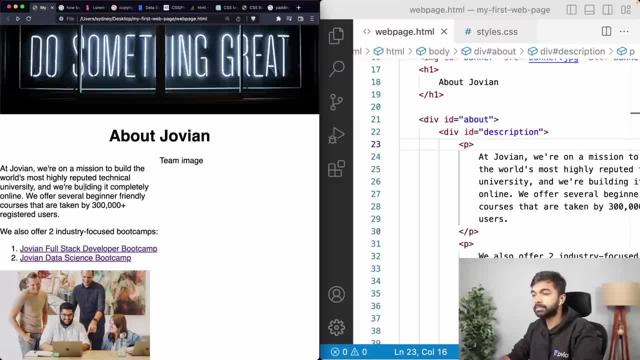 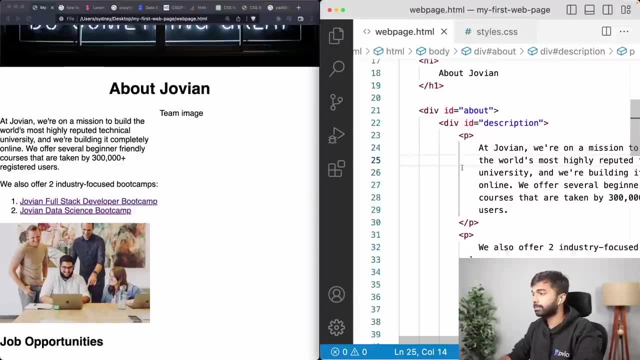 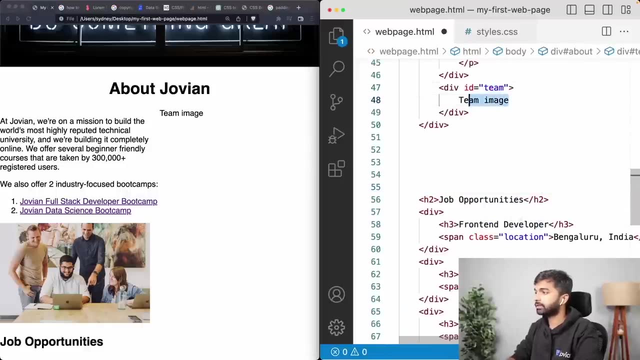 It should be formatted already And now you can see that this P tag contains the data or shows. this P tag shows the information on the left half. Similarly, we can take the image now: This contains this, the team image, and we can put that here in the team section. 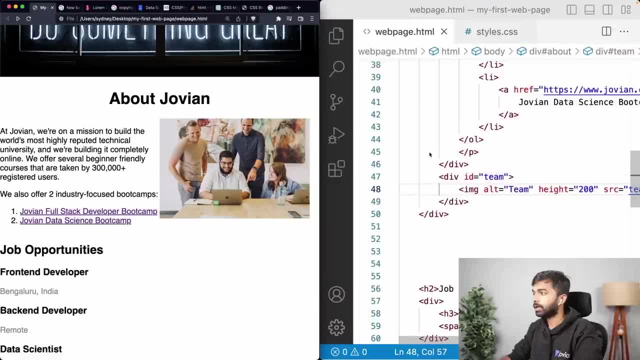 Okay, now we have the team image on the right. Alright, so that's one thing that I want to point out to you, that you should. what you should do is you should first try to create a layout Using a couple of empty divs, maybe even add background colors and borders to them. 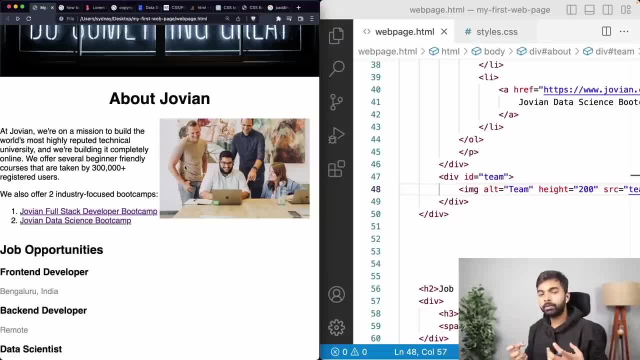 just so that things are super clear. And once you've created the layout with those empty divs, especially horizontal layouts, then put the content inside, because otherwise you might just lose track and become confused. But now, once you put the content inside later, you have actually already fixed all of this. 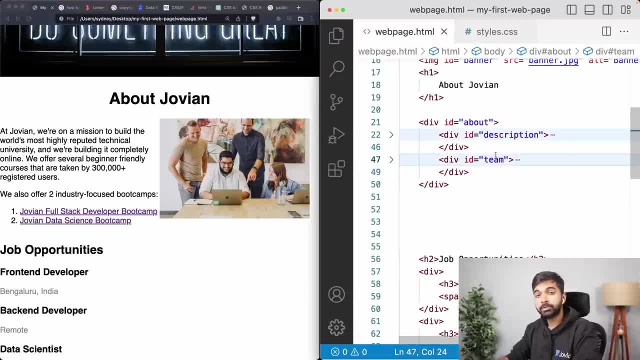 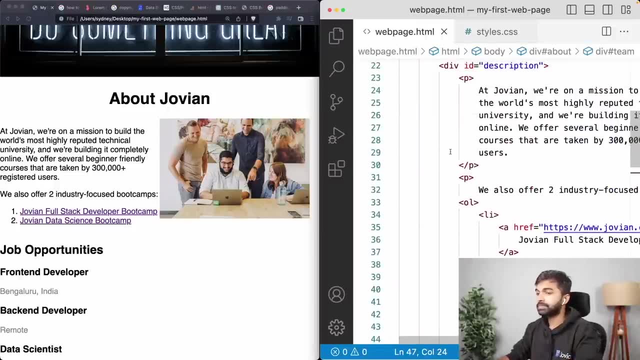 So you're fixed what the description and team should be laid out as, and then the content inside can be laid out independently. Okay, So build your web page step by step in these steps. Okay, let's maybe clean this up a little bit further. 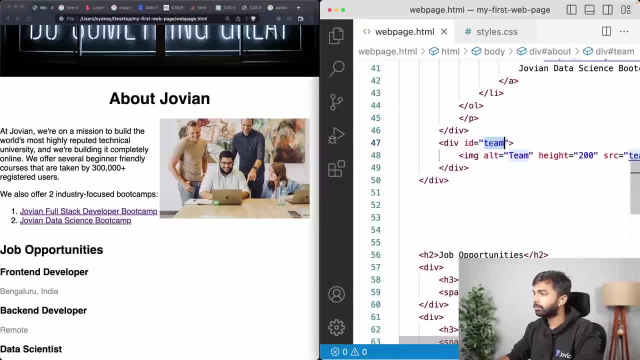 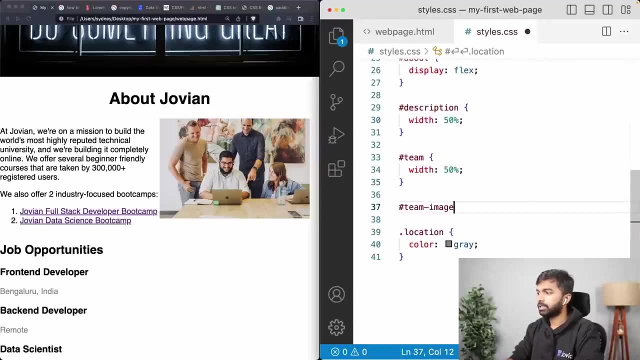 Let's see. So maybe this team image, this can have a border radius, So this is looking too sharp. Let me just call: give this an ID Team image And let me come in here: Team image and let me give it a border radius. 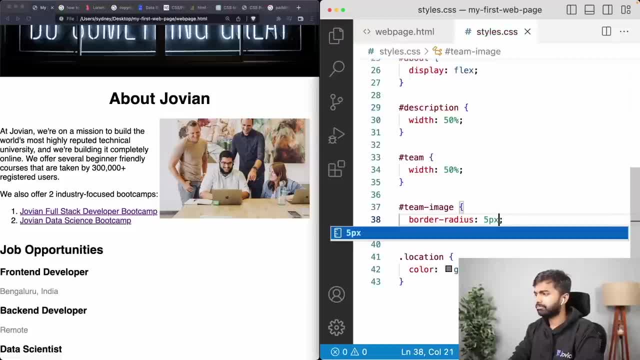 Let's give it a border radius of five pixels- Again, experiment with a trial and error, but yeah, five pixels looks good. I think I would like to have maybe some space here, So maybe I can go in and I can add some padding into team. 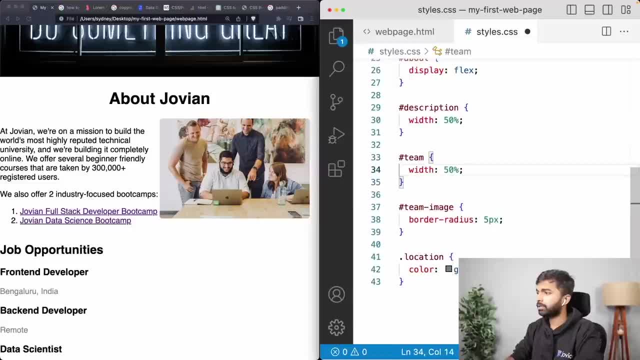 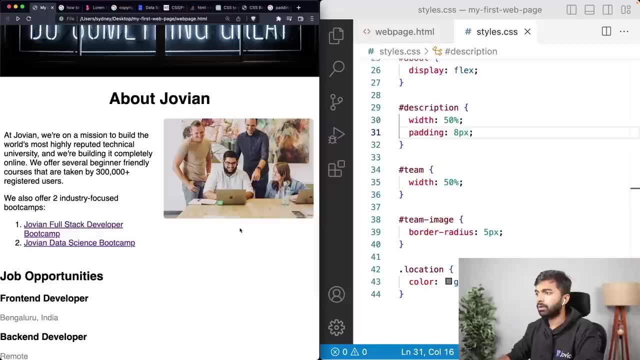 So let me come into team and add, or let me come into description and add some padding. Let me add a padding of eight pixels. Okay, So now I've added a padding And maybe let me add this padding only on the left and right. 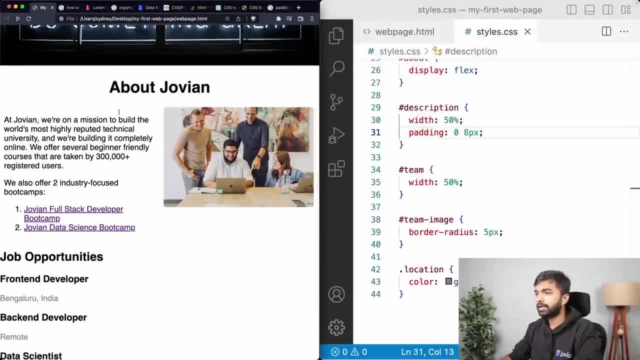 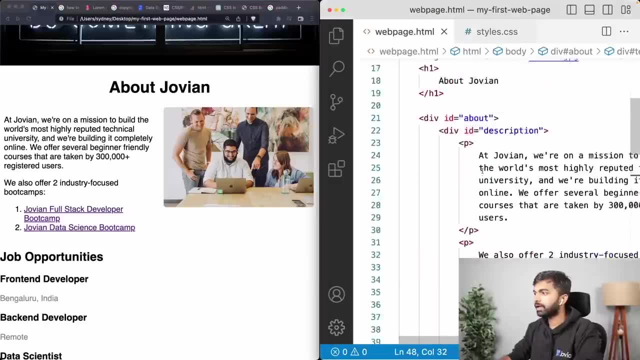 So let me keep the padding top and bottom as zero And let me add that padding. But you can see here that there seems to be some space above this as well, And I believe that is because of this paragraph tag, Because this paragraph tag generally has some space above, and I can verify this by creating. 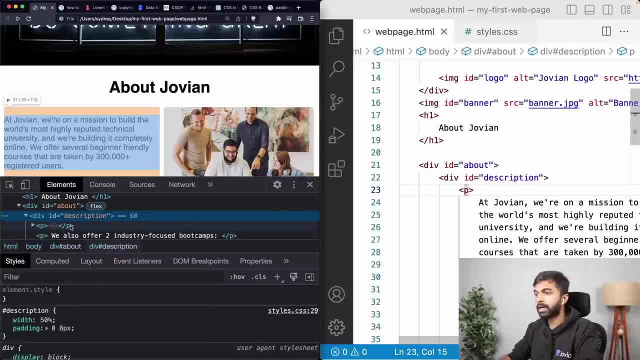 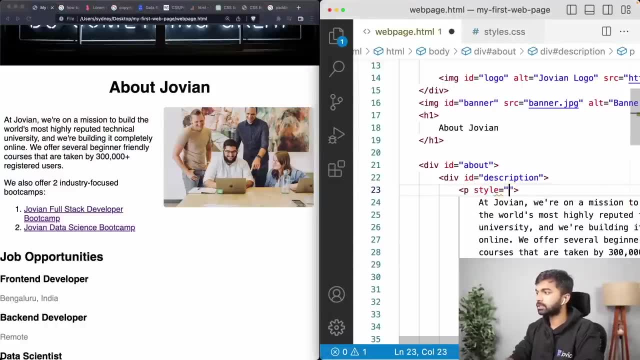 is by clicking inspect and verifying that in description. this paragraph tag has a margin above. So I can just set for this particular paragraph tag style equals margin zero or margin top. When you're specifying a zero margin, you don't need to say px, you can just say p margin. 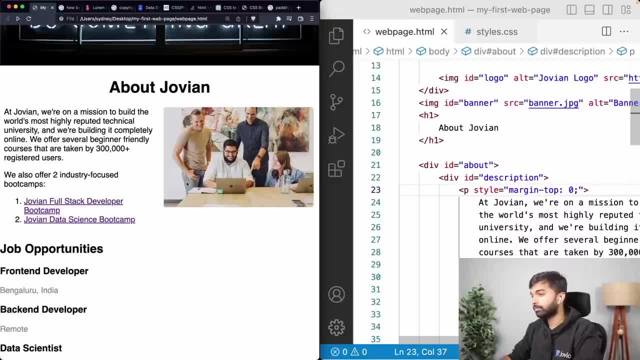 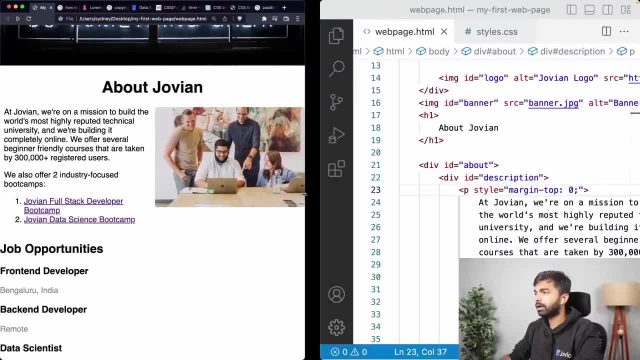 Okay, great. So the page is starting to look pretty good. I would say One issue here is that if I extend this forward, looks like I have a for this team image. looks like I have a width set. let me get rid of that width here. 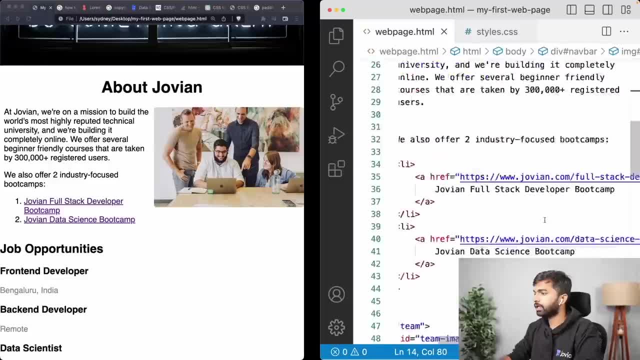 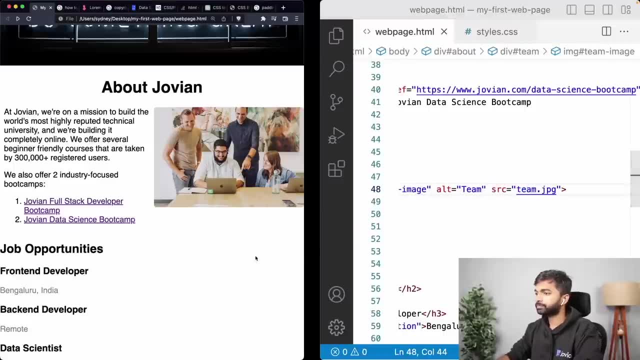 Or a height. Okay, Okay For the team image. where is the team image over here? Yeah, this is a team image. I think I have a height set for it. Let me get rid of the height that I've set. 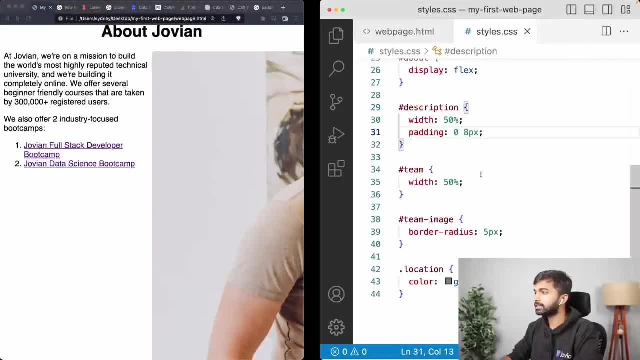 And now it ends up taking up the entire space. So maybe what I can do is I can just come back in here under team and or under team image and I can set the height to. I can simply set the width to 100% of the parent. 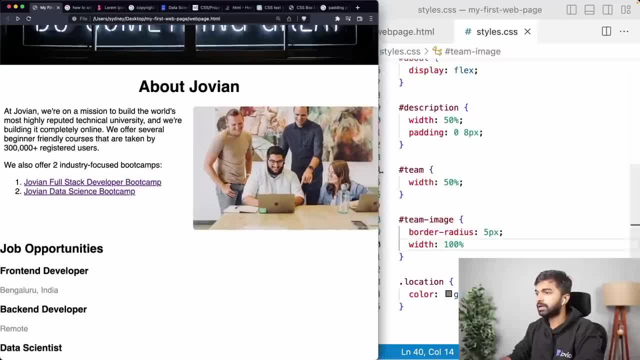 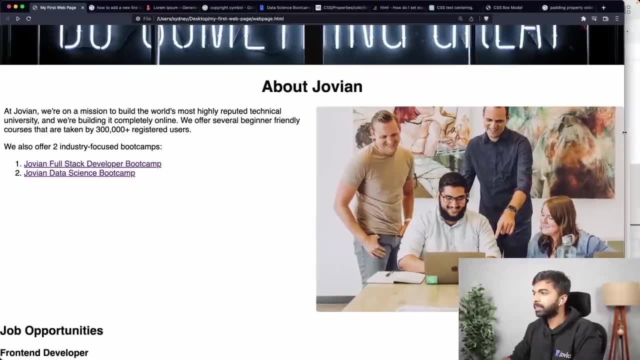 which is half the div. Okay, So that's nice. Now it is taking up the entire space inside the inner div. Okay, So this is expanding in size based on that. But as the page gets bigger and bigger, this content becomes too wide. 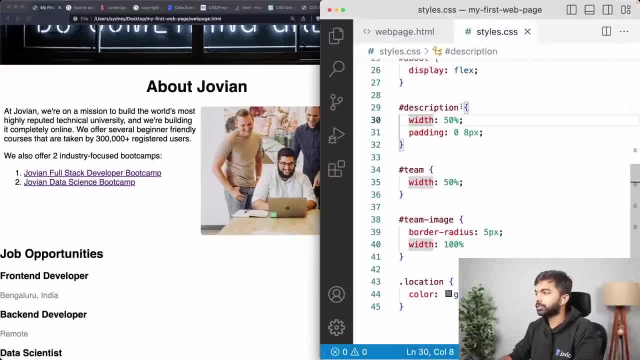 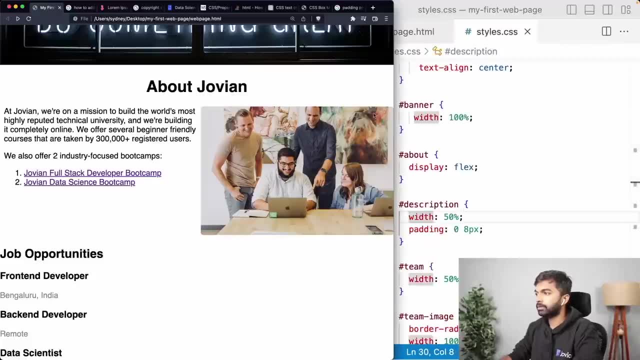 So maybe I want to limit the overall width of this description, right So? overall width of the About section itself, right So the About section. I don't want it to become too big, The About section should. maybe I do. I just want to restrict it to this region generally. 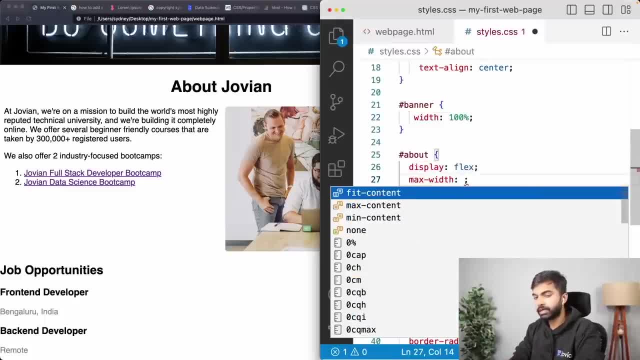 speaking. So what I can do is I can set a max width. I can set a max width, or the max width is the maximum width that this particular section should have. Okay, So this is the maximum width that this particular section can take. 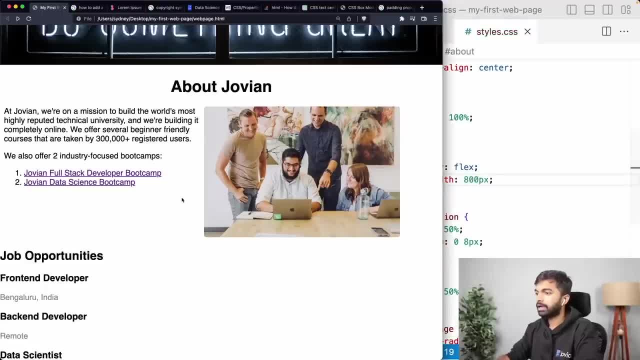 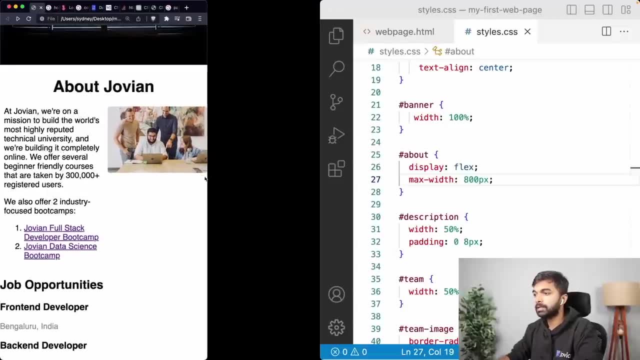 So max width: let me set it to 800px And let me reload the page. Now you can see that even as, as we make the page smaller, both of these are going to take half the space, And as we make the page bigger, it's going to stop at 800 pixels. 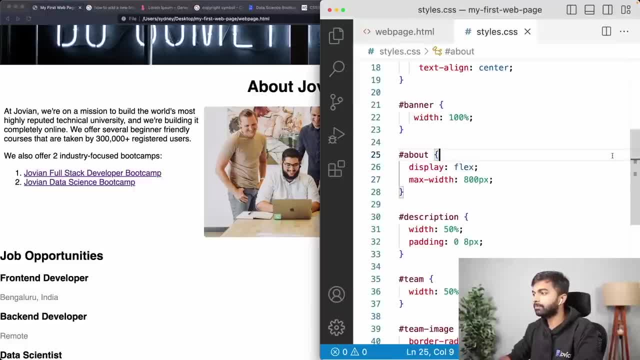 But of course it would be nice for this to be centered on the screen. So that's where I can also use that margin trick. I can say margin zero, auto, zero margin on the top and bottom, And then right and left margin can be auto. 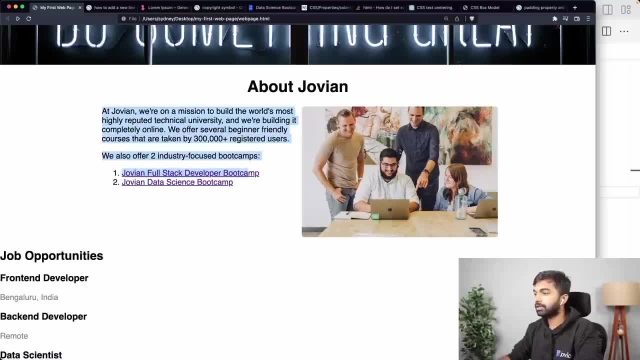 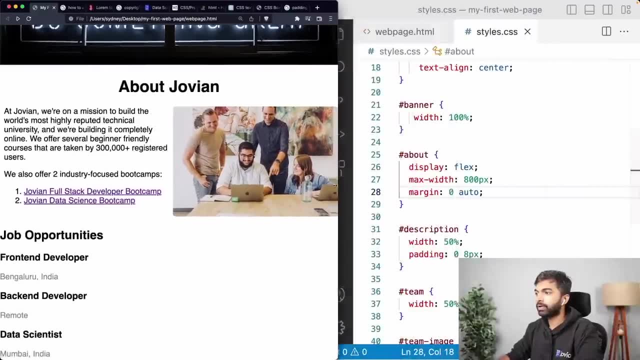 And now you can see about German, and here we have this, and then we have here we have this image and it's all nicely centered. Okay, so remain centered, remain centered. and then it goes out here and it becomes small. Okay, and maybe we can also add some padding here. 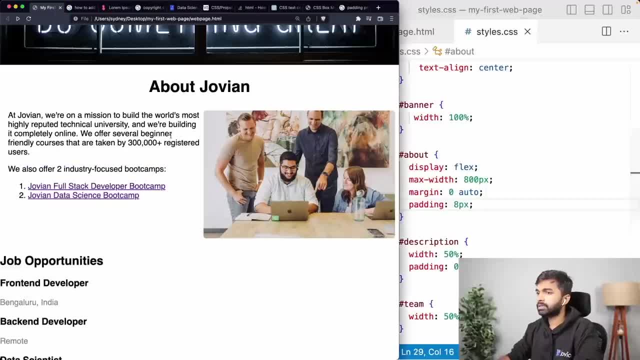 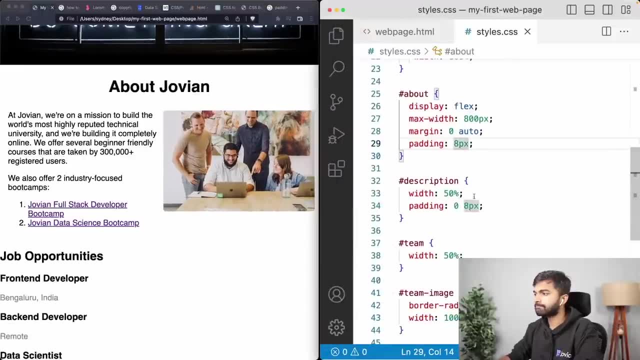 Let's see, let's add a padding of maybe eight pixels just so that it's it doesn't touch the edges. Okay, And if you've added padding here, then maybe we don't need this padding here over here, maybe we just need a padding, right? 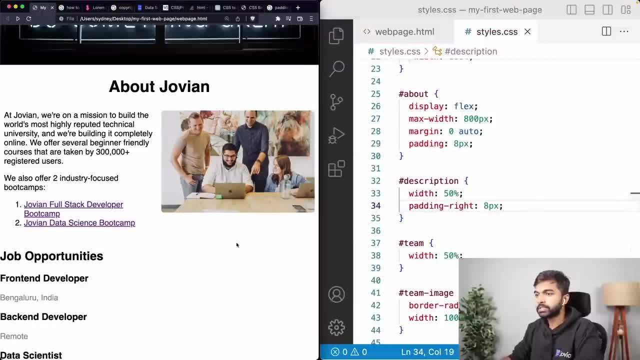 Eight pixels. Okay, so this is what web developers sit into all day. they fiddle around with small CSS settings just to get things to look exactly as they desire, But this is looking fine to me. I think the About section looks good largely. 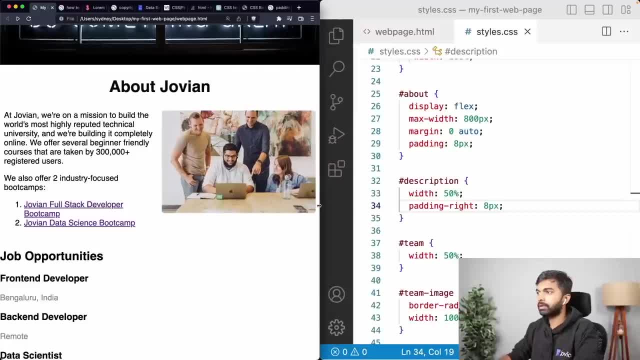 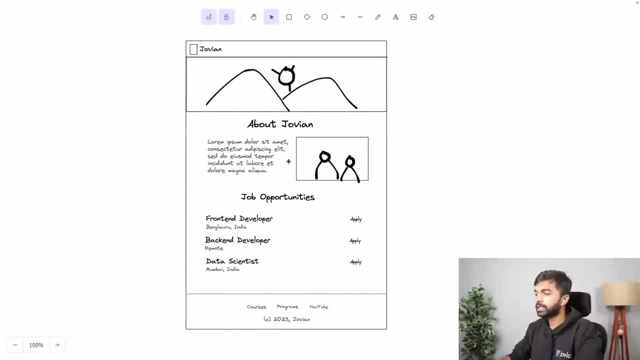 Yeah, somewhere around that is looking good. Yes, this is slightly falling over into the next outside, but that's okay. Okay, So now we're done with the About Jovian section. let's go ahead and fix the job opportunities section. 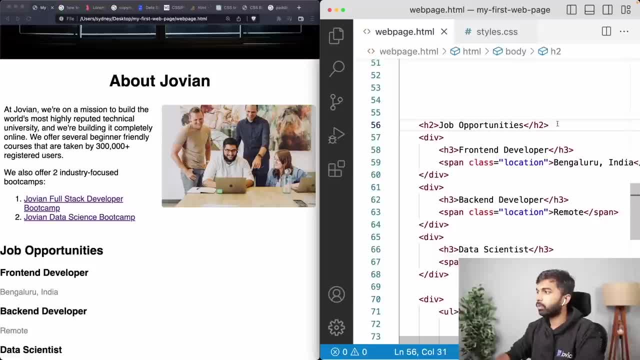 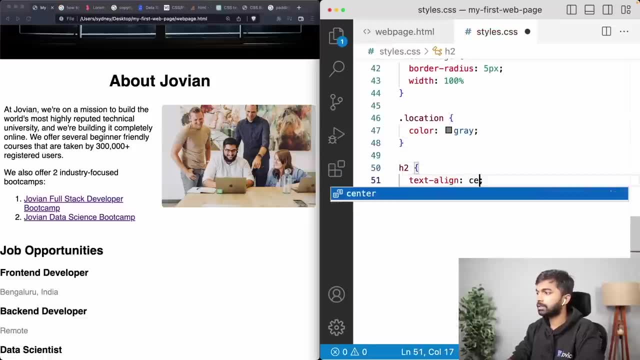 So I'm going to go in and under job opportunities, okay, once again the H2 as well. I'm going to add a set center, So H2, I'm going to say text align, enter. okay, now this has centered, then I can go. 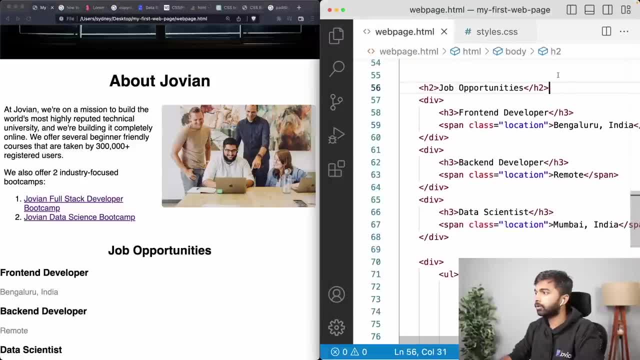 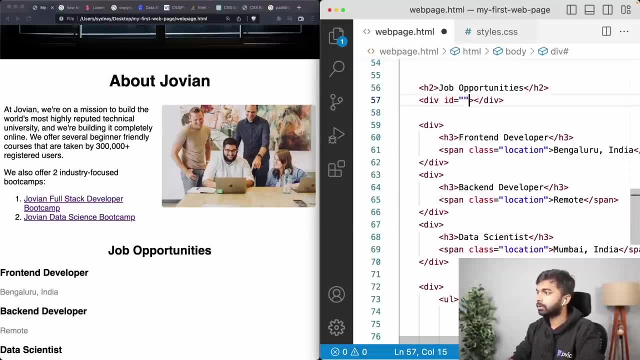 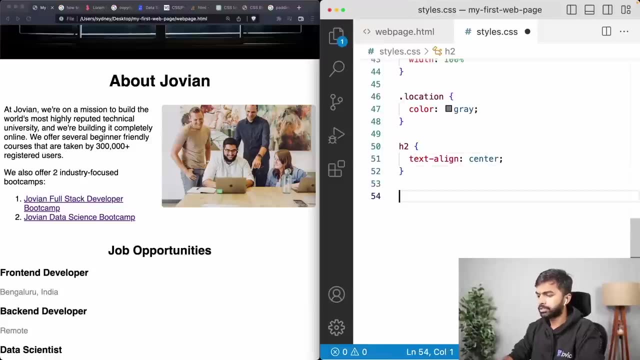 in and I can maybe again create another outer div called jobs. So I created a div called jobs, So let me give it the ID jobs. All right, And again for jobs, I'm going to set a maximum width. The max weight for jobs is 800 px. 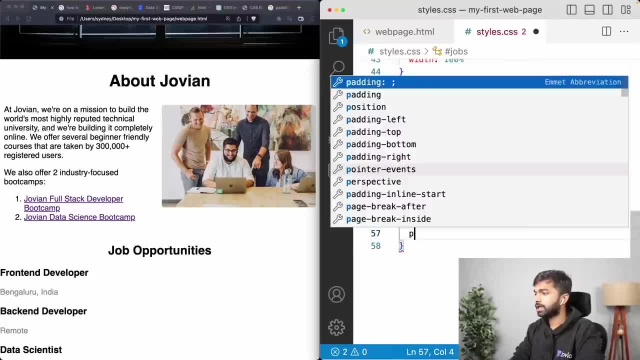 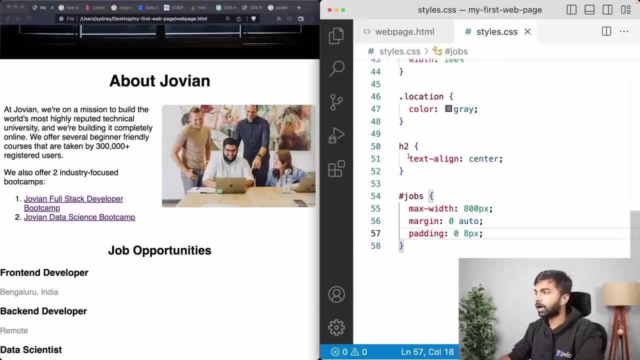 And I'm going to set margin zero auto. I'm going to set adding zero eight px. Okay, all I'm doing is I'm creating an outer div into which I can add a div Okay, Which I can then put in all my jobs. 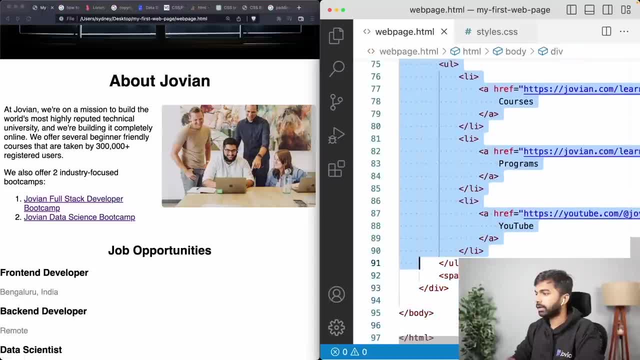 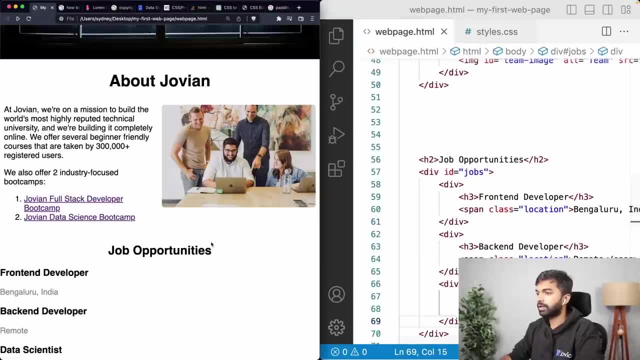 Let me grab all these jobs. And this is all the footer. Yeah, all this point. to this point. we have the jobs. I'm going to put it under the jobs div And let me reload again And you can see that it has this. nice, it remains centered on the screen. 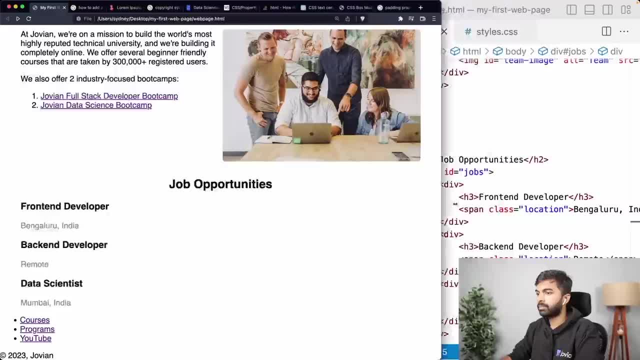 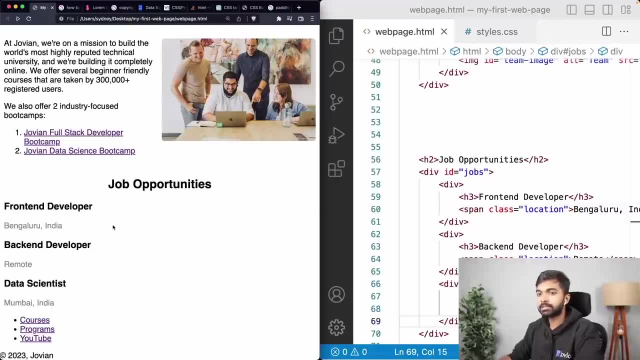 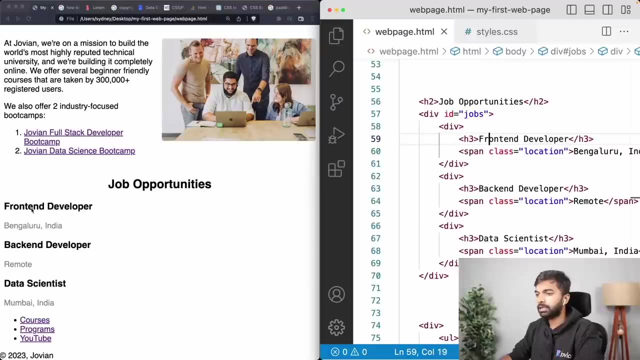 That's nice, Pretty good. Remains centered on the screen And it is also not touching the edge of the screen. So generally you want to have some space from the edge of the screen here, So that's it. Okay, then we have this h3 over here. there's a lot of space between front end developer. 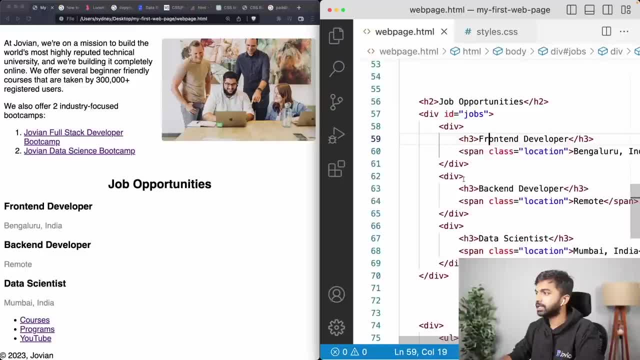 and then Bengaluru, India. how about we come in? this is an h3, remember it's an h3. Let's give it a class called job role, so that we don't affect other s3s on the page if we. 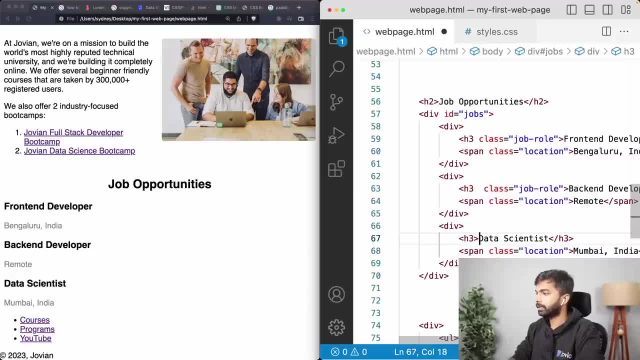 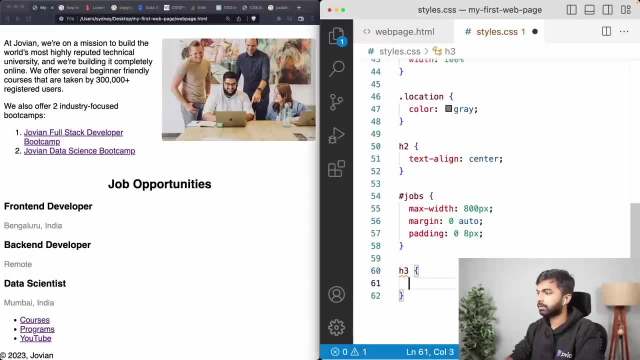 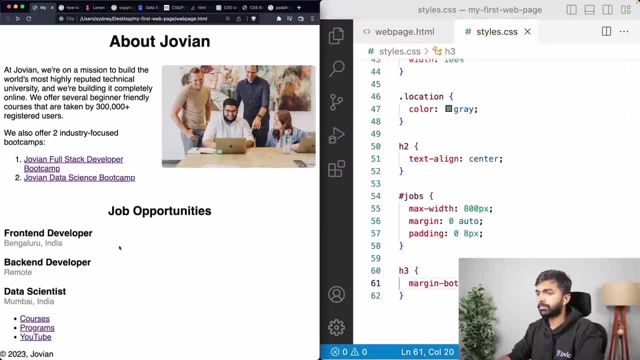 had any. at the moment we don't. But yeah, Okay, And let me come in here h3. And let us just give it margin bottom zero. I believe it's a margin. Let's see. Okay, margin bottom zero. this is looking good. 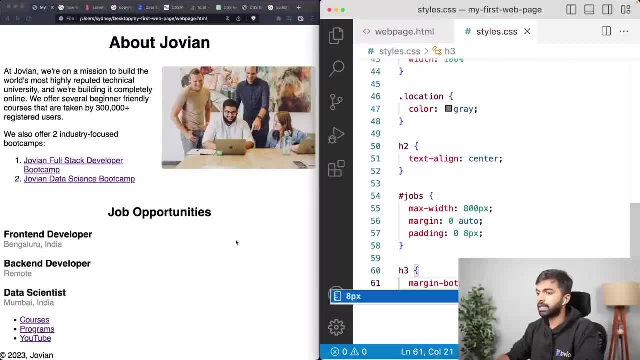 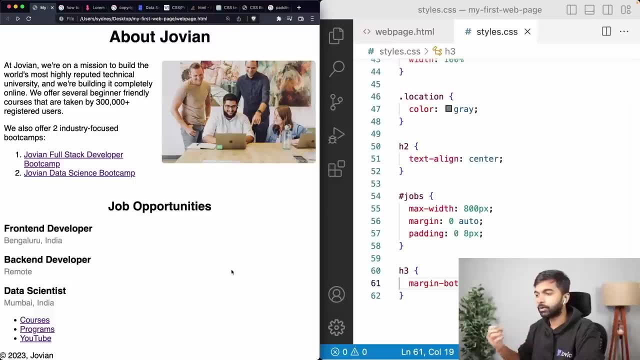 Now it is much closer. maybe zeros too little, maybe let's make it eight px, maybe four px should do the job. So normally, with margins and paddings, you want to use multiples of four, that's a good idea, And you want to go double, double, double, half, half, half. 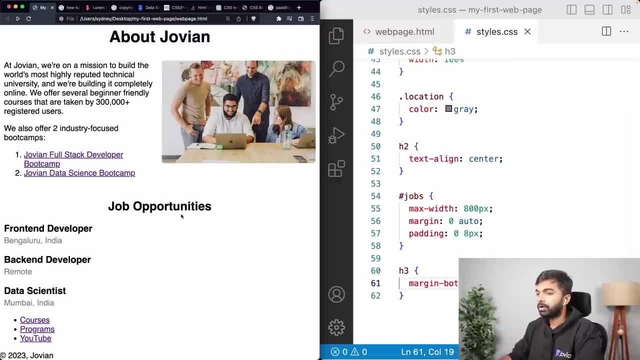 And that's a quick way to work around this stuff. Okay now, what would be nice if we could also get that nice apply button or apply link here on the on the job page. I'm going to again show you a quick trick. we're going to learn a lot more about things. 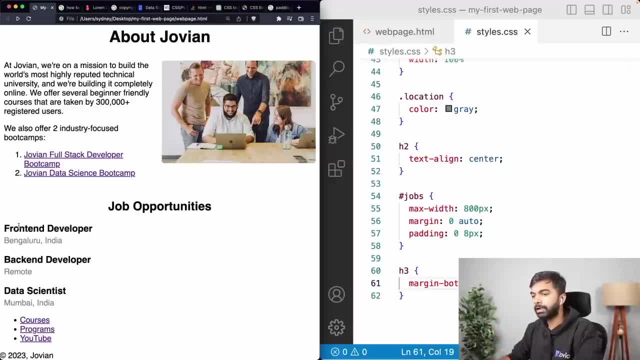 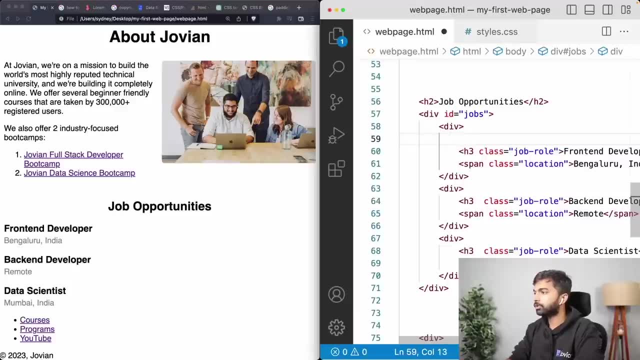 like flexbox etc. But a quick trick to just get one single element pulled to the right side is using something called a float. So I'm going to show you right now. So let me say: a href equals nothing for now, And let me just put in: apply. 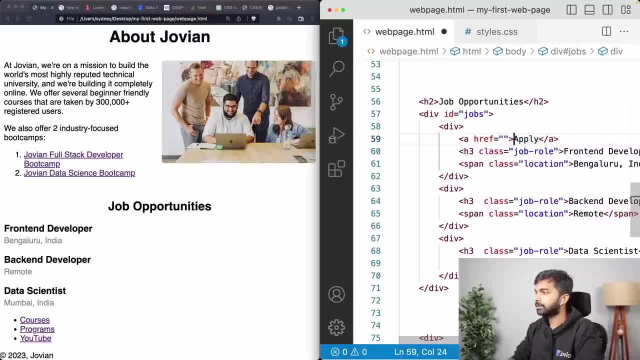 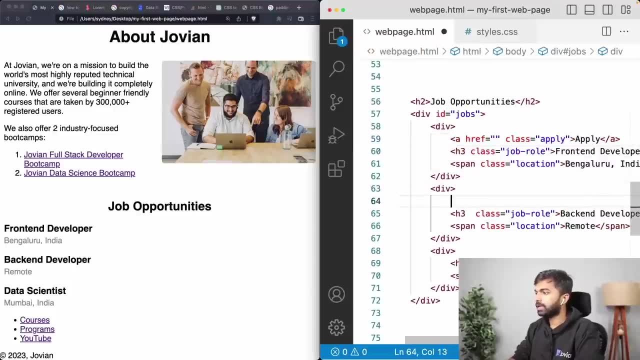 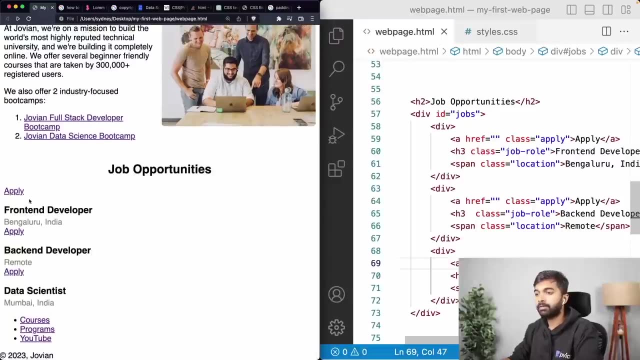 And let me give this a class as well, And this class is also called apply, And let me put it above every h3 here. Okay, so now we have this: apply, apply, apply. that is going to show up above every h3.. 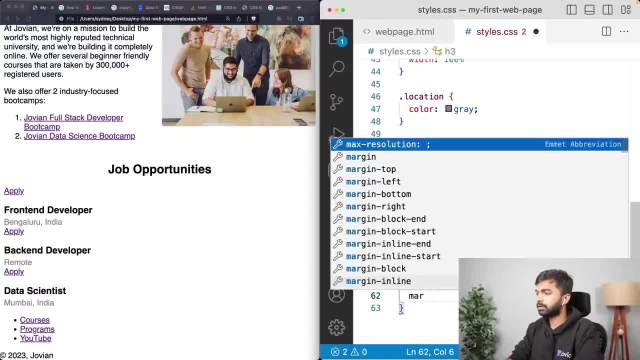 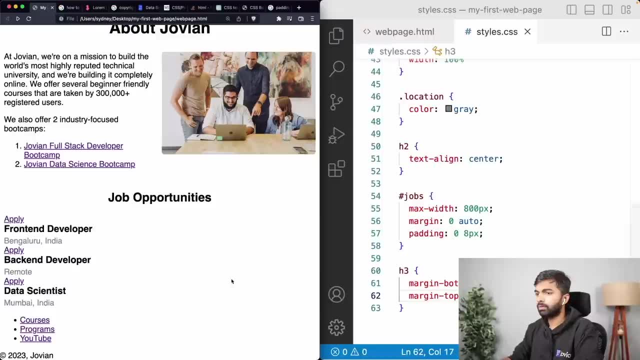 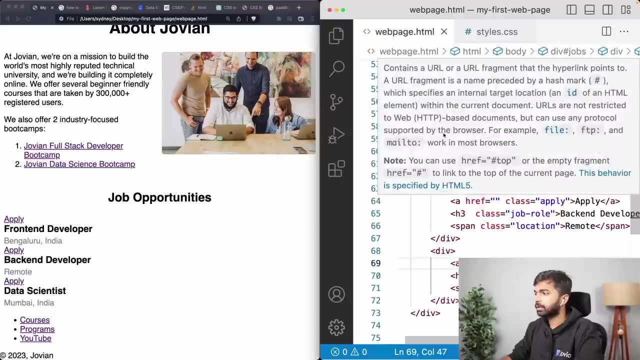 And I think I can go in and I can fix the margin top as well for this h3 to be zero. Yeah, so now we have apply, apply, apply, And what we can do is take the apply class. so, dot, apply. that is the. that is a class. 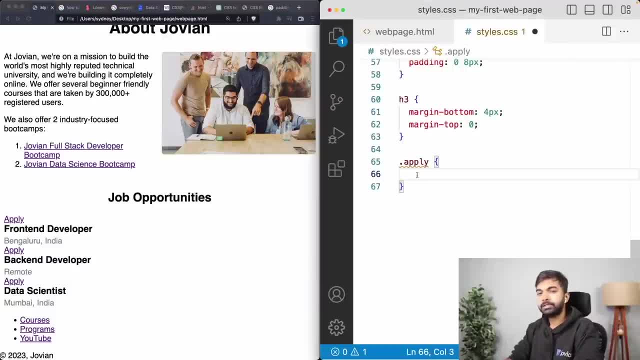 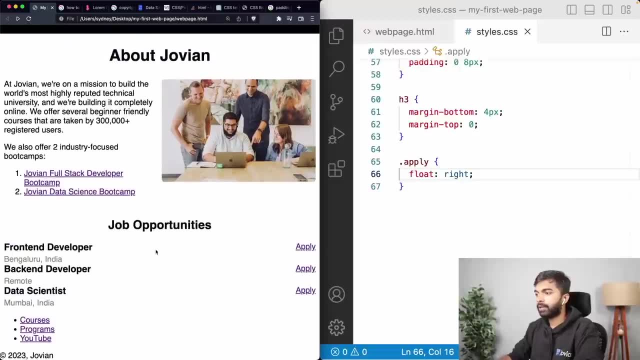 given to this apply link And I'm just going to add one thing: float, right, okay. So that's just going to pull this apply all the way to the right. That's nice. It's going to just pull it all the way to the right. 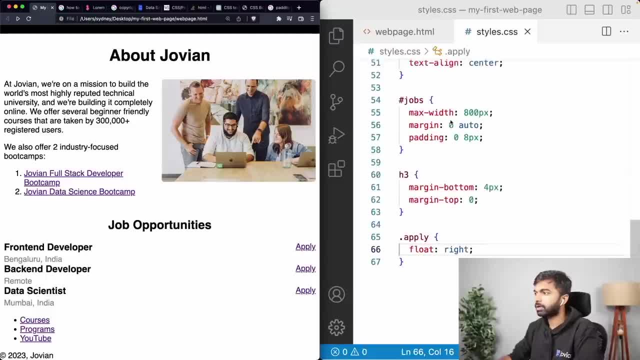 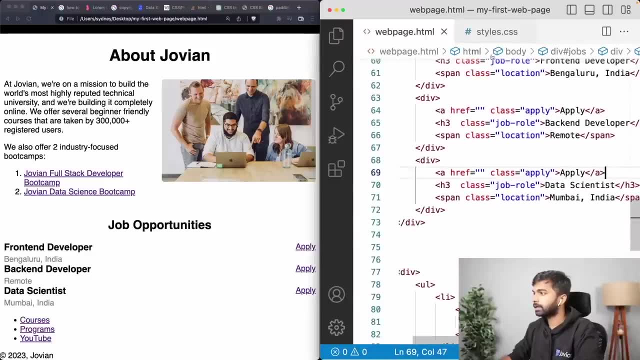 Right And you can see under the location, we need some spacing So I'm going to go back and add some location. add some spacing under location. So we have class location And class location has already had. we've added the color gray. let me add margin bottom. 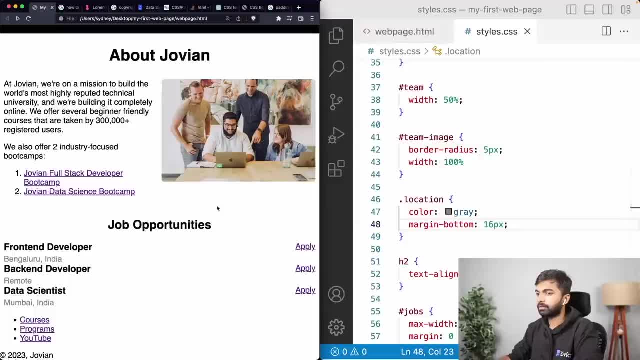 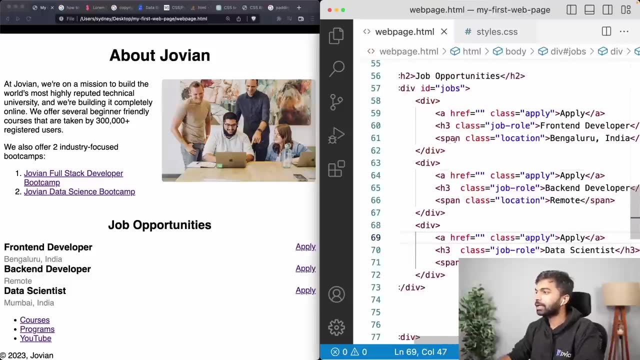 16px. Okay, that's a span, So that's another learning. margins don't work for spans. I know it's confusing, Happens all the time. Okay, Margins don't work for spans, So I'm just going to go in and I'm going to change these spans to divs. 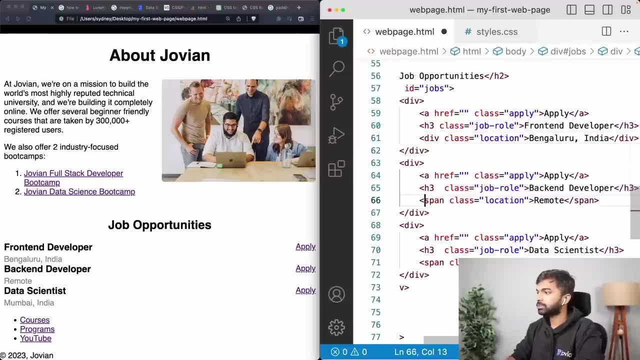 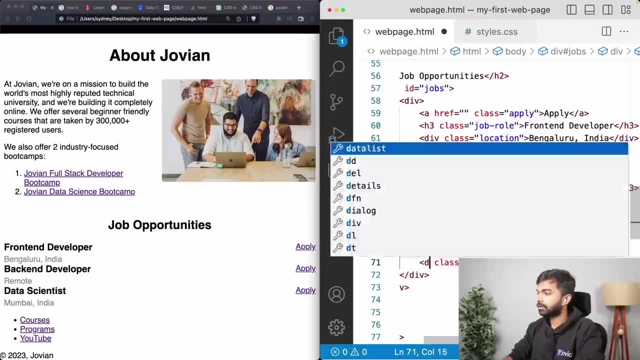 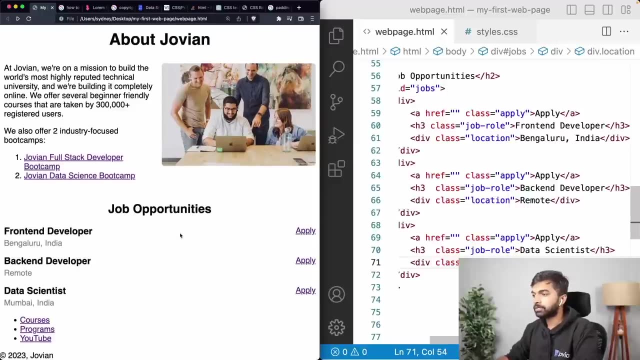 Okay, Margins and paddings don't apply to spans because they're inline elements. I'm going to change these all to divs And now it's going to apply. Okay, great. So this is looking nice. Now we have the front end developer, we have Bangalore, India, and we've pulled this already. 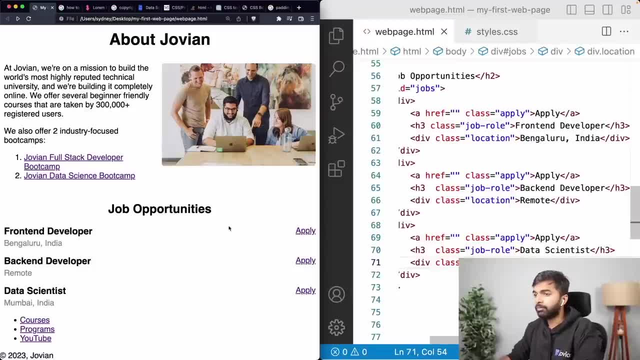 floated. We have the back end link to the right, So that's nice. One thing that I would want to do now is maybe get rid of these underlines under these links. These underlines aren't looking that great. I'm just going to go in and then, for all the anchor tags, I'm going to remove the underline. 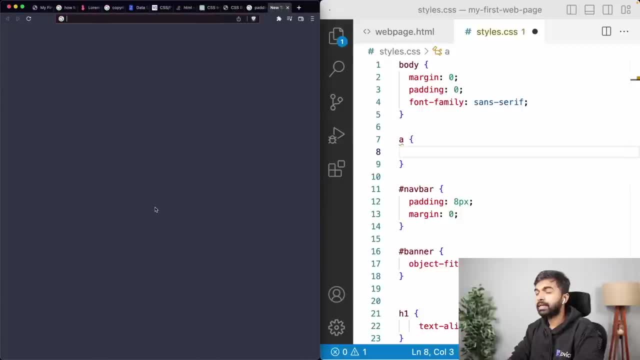 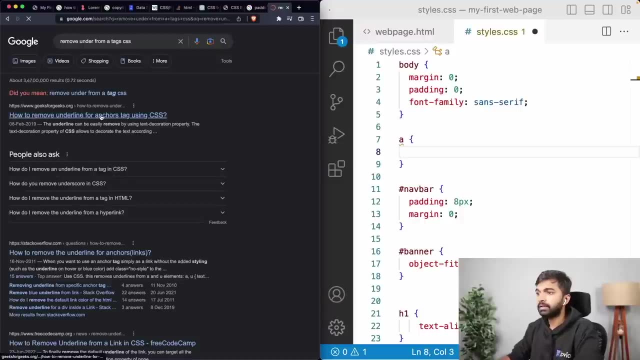 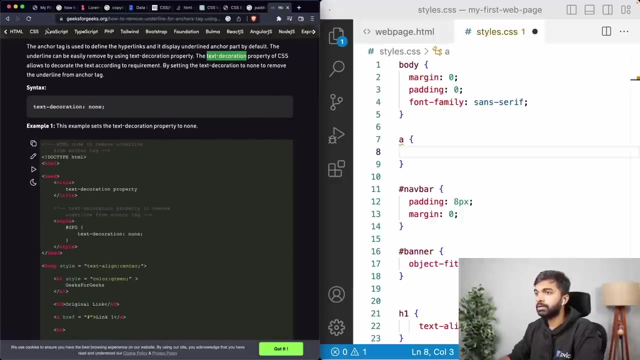 How do you remove the underline, all the anchor or the link tags? Well, remove underline from a tags CSS. I just search that And it says that it can be removed using the text decoration. Okay, So you can say: text decoration: none. 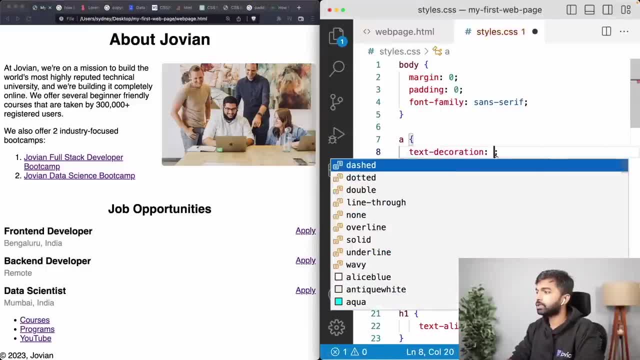 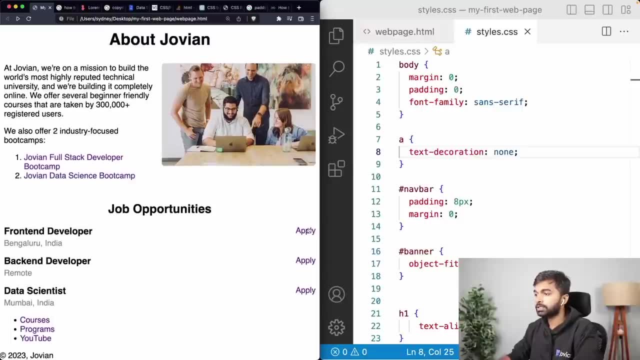 And that should do it. If I go text decoration, none. that should hopefully get rid of all the underlines. right, We have gotten rid of all the underlines as well. Now we have these apply links as well. Last thing is the footer. 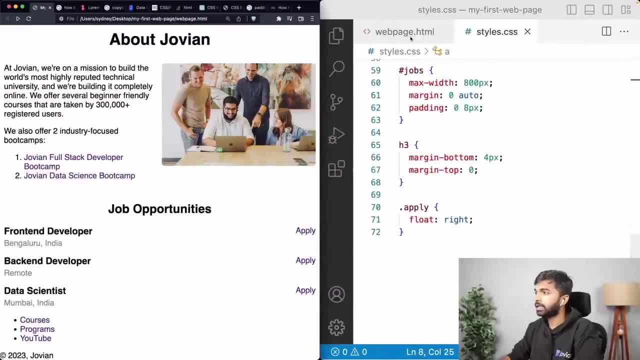 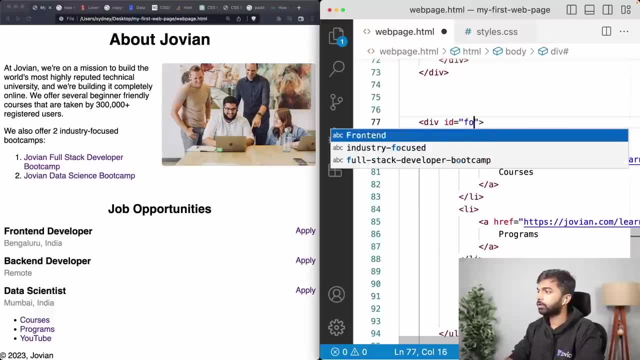 I think we're almost there. We just need this footer at the end. Let me come in And, once again, let me create this div called footer. Okay, it's already there, So I'm just going to give it the ID: footer. 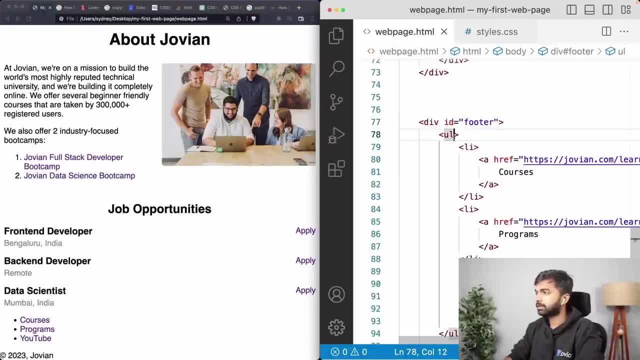 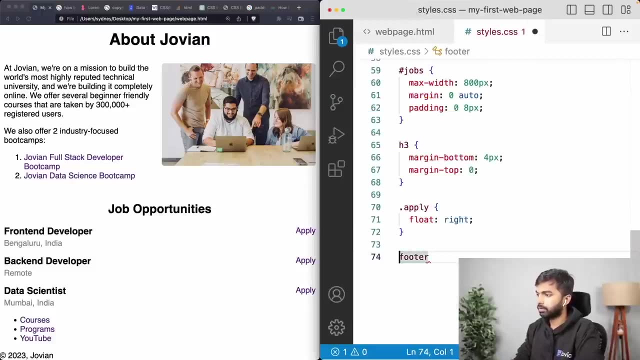 Okay, And then we have this list. Let me just call it, Let me give it the ID: footer links. Okay, so I'm going to do a couple of things. First, I'm going to give the footer dot it's, it's an ID. 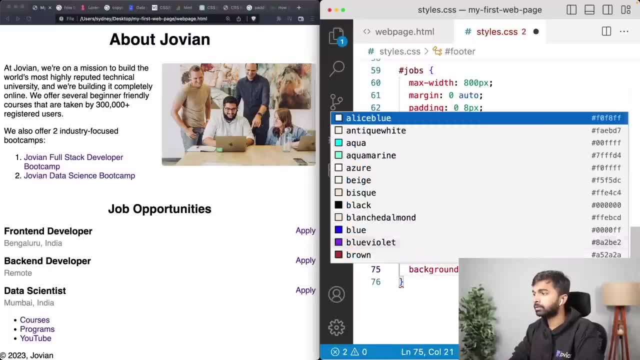 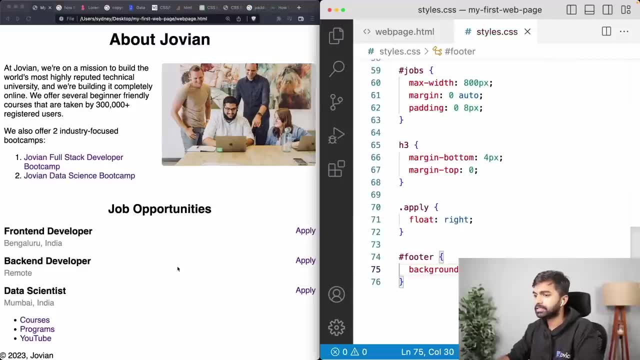 So hash footer, I'm going to give it the background color, gray or something very light gray. Let's see Underiro, look. Okay, that looks like a nice grayish color. Oh, what is the lightest gray we can find? 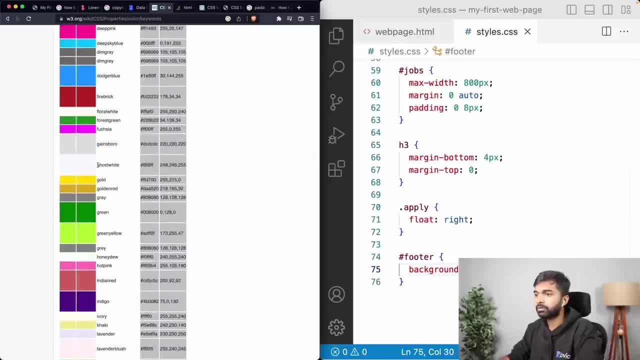 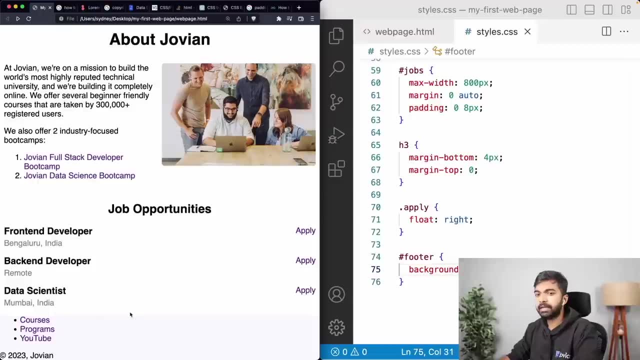 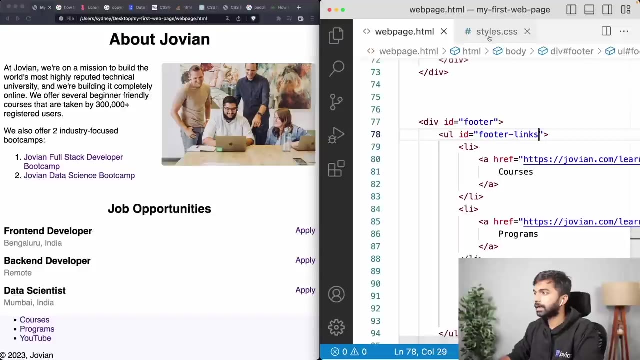 Let's search for a very light gray, ghost white. Okay, that is interesting. Let me just get ghost white. Yeah, that's a very light grayish color. you may not even be able to see it on the screen, But it's there then, or the footer links. I want to get rid of these bullet points. 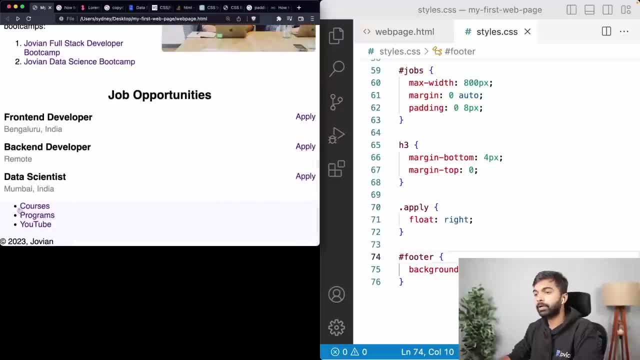 And let me just bring that up here. So for the footer working links, I want to get rid of the bullet points And I just want to keep them all on the same line. So I am going to say footer links And again, this is something that I would look up normally. 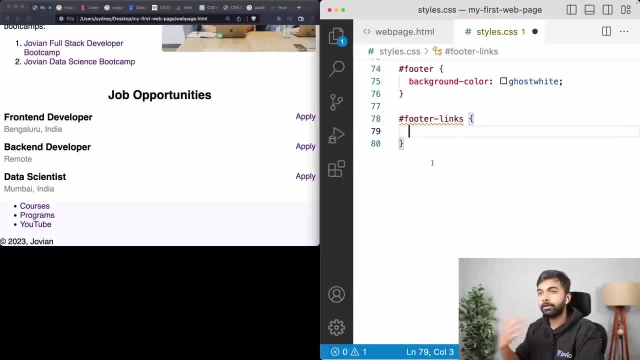 but I happen to remember it, What the way you can get rid of these bullet points is to say, list style none. I believe that should do it, And now you can see that the bullet points are gone. Of course, for the footer itself, it might be nice to maybe add some padding. 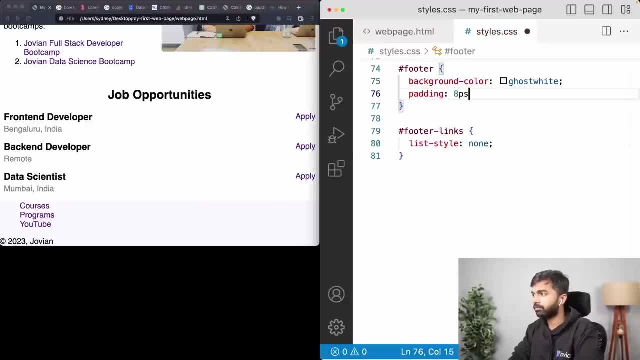 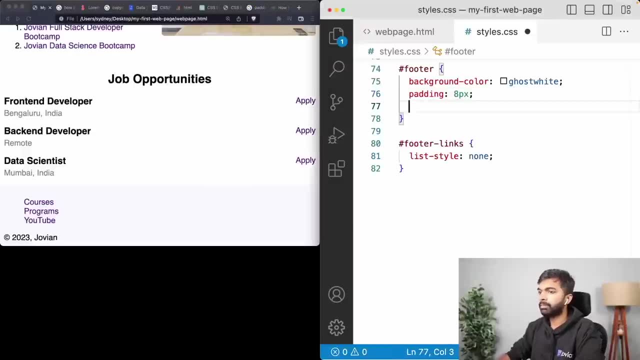 At the top and bottom and maybe all around. So let me just add a padding of eight px And okay. now the footer is looking nice too, And maybe let me also add some margin top. the footer is too close to the data scientist job role. Let me add a margin top. I'm going really 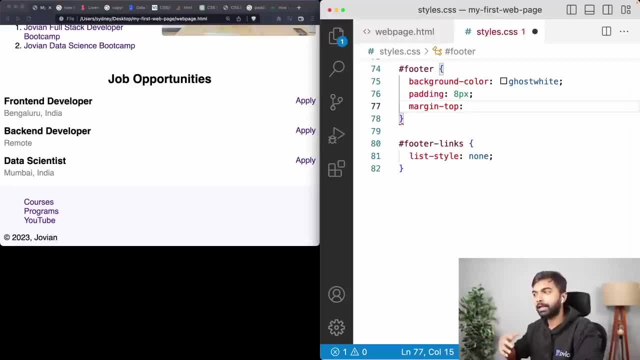 fast, but I'm expecting you to follow along here, pause, follow along and maybe also look up what each of these properties mean, because that's really how you do web development: 16 px. So let's add a margin And let's see. 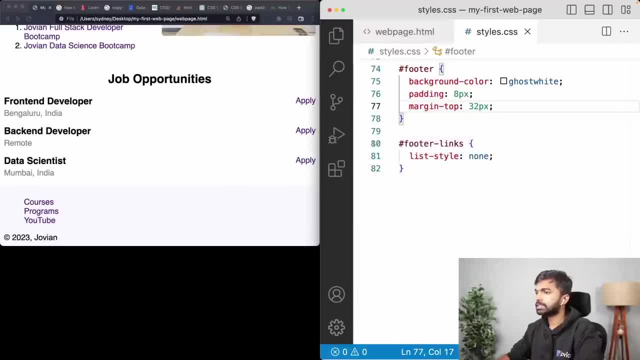 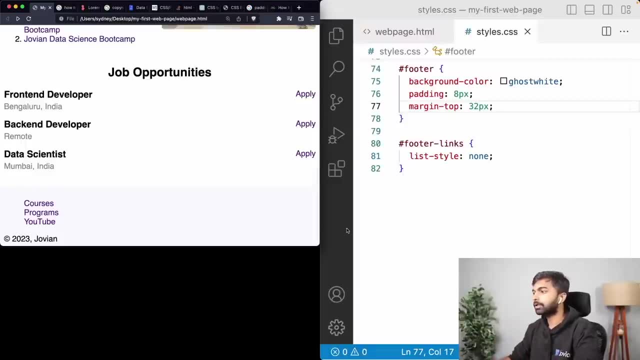 did not do anything. Maybe let's make that 32 px. Yeah, not increase it. So remember our location also has a margin, So the margins collapse into each other. All of that happens, Okay. final thing: we want to make these list items come up in line, So there. 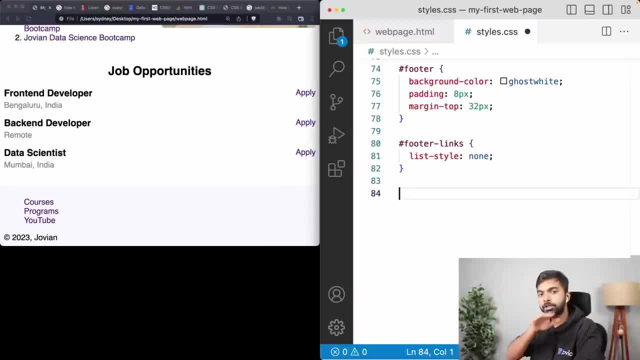 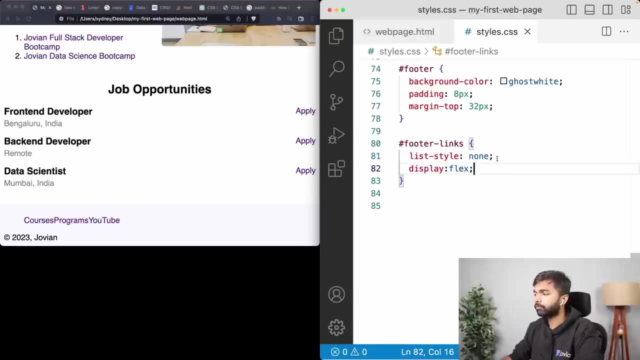 whenever you have three divs showing one below the other and you just want to show them all in line. Now, another quick way to do it is: well, we could just do, I think, display flex, and that would do it. Yeah, display flex, and that should do it. For footer links, we can also add: 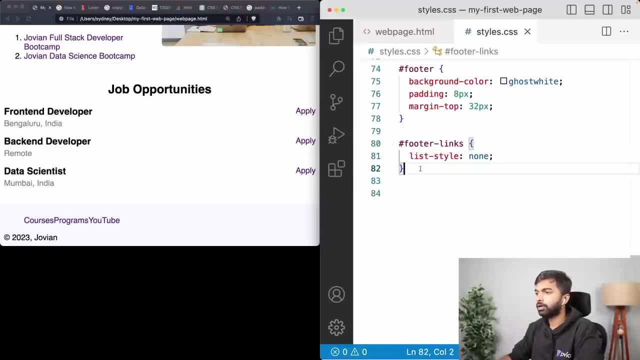 But I want to show another way to do it And this is something that you can set on individual list items So you can see footer links, li, And that is going to select the li items under the ID, footer links, And I'm going to say display inline. 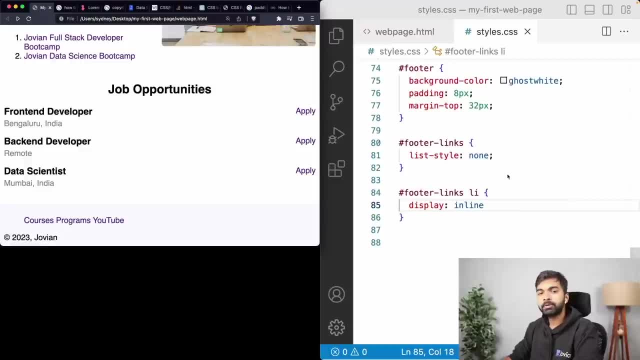 Okay and you can see now they're showing up inline. So the difference between flex and inline is: flex is something that you apply on the parent And that applies to all the items within it, And then inline is something that you apply to the child element. let's say you went into one of 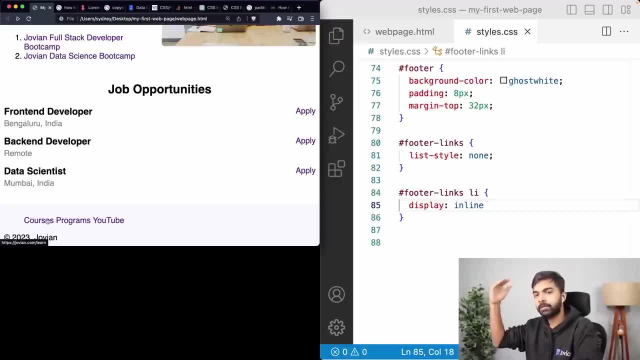 these list items and applied inline only that would appear inline instead of block, which is the entire horizontal width. But here we are applying to all the list items And I'll tell you why in just a second. But apart from the inline, we also want to add a margin. So let's add: we don't need a margin at the top. 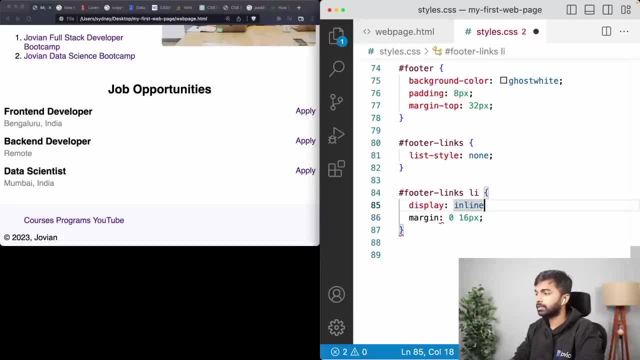 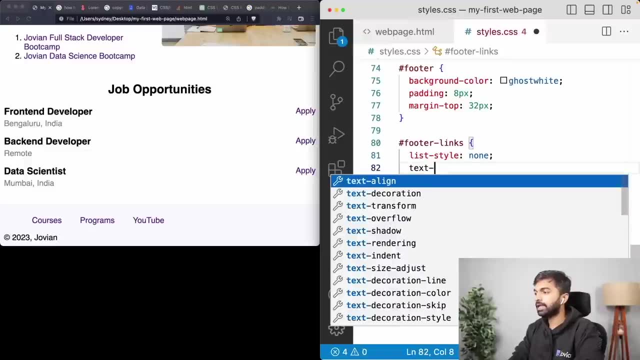 let's add maybe 16 pixels of margin on the left and right. So let's add the margin here. Let's reload, Okay, so now we have a margin, And the last thing I'm going to do is I'm going to say text align center And that is going to center these links on the page. Okay, And in fact, 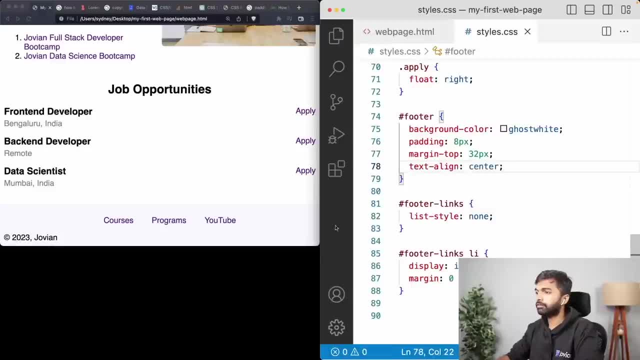 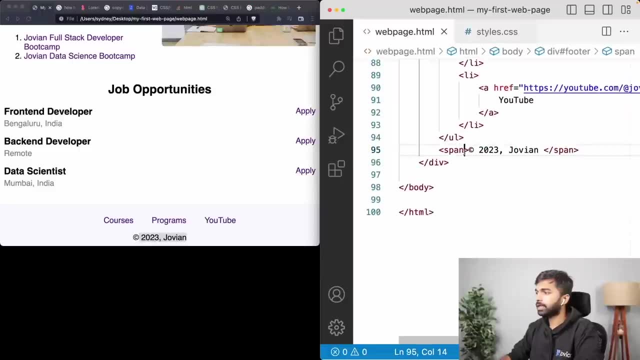 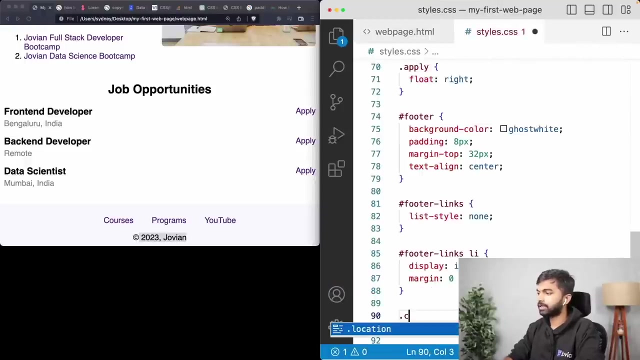 text align center can be done not just for footer links but for the entire footer links, So we can do it like that. And finally, let's fix this as well. So let's go in and let's call this copyright, class equals copyright, And let's come back in here. And well, we could also give it an ID. but fine, classes, fine. 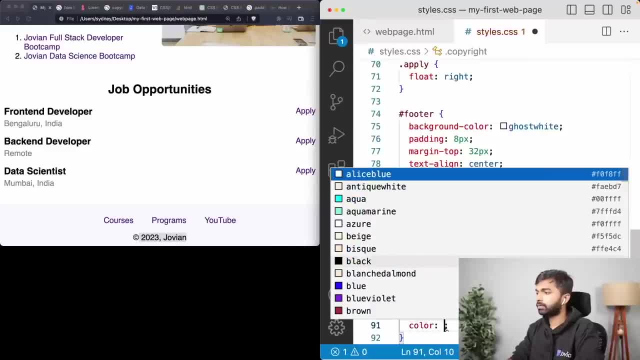 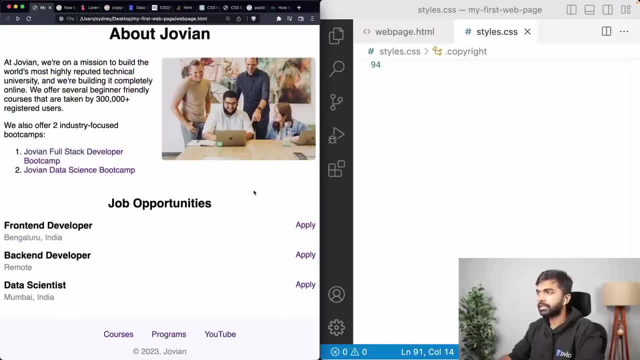 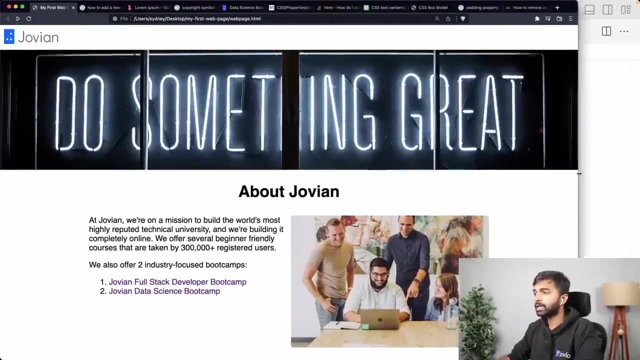 Copyright and let's give it the color gray. Okay, so that is our page. I think that is looking pretty good. So we have the nav bar. at the top, we have this banner, and this banner always occupies the entire length and it doesn't stretch the image too much. Then we have this about German section, that 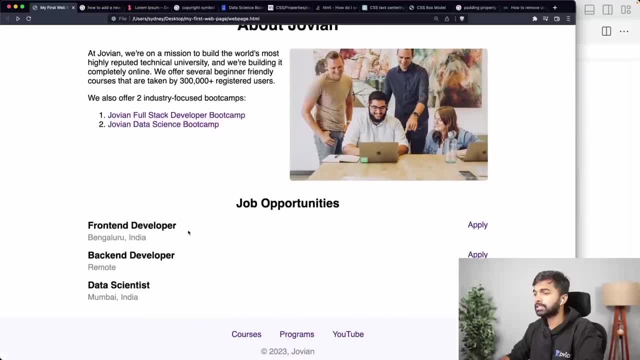 is always at the center, And then we have the job opportunities that are also in the center. If you want, we can experiment with the colors of these. And finally we have these apply links. They don't do anything right now, But it wouldn't be nice if they could at least. 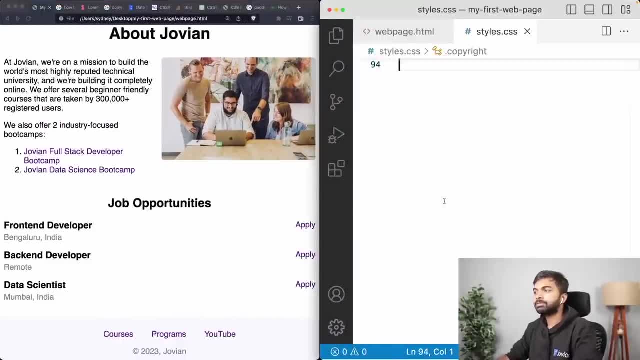 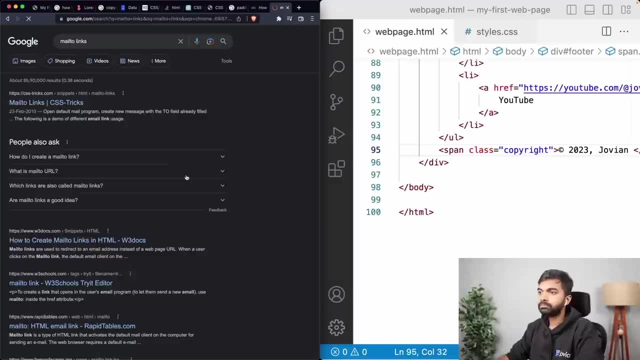 trigger some sort of an email, And that's where I want to introduce you to another form of link called mail to links. Okay, we just searched for mail to links. What is a mail to links? Well, you can do this instead of having a link point to some. 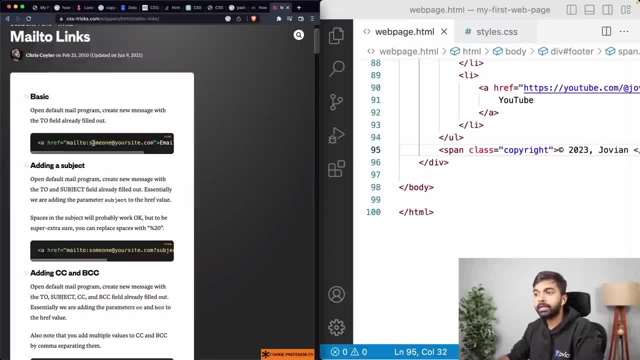 website on the internet You can have a link, say mail, to colon and then some email address, and when the user clicks on that link it is going to open their email application. whether it's Gmail or whatever email application they're using, it is going to open their email. 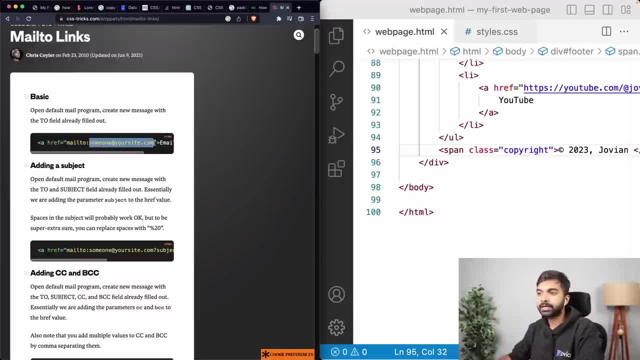 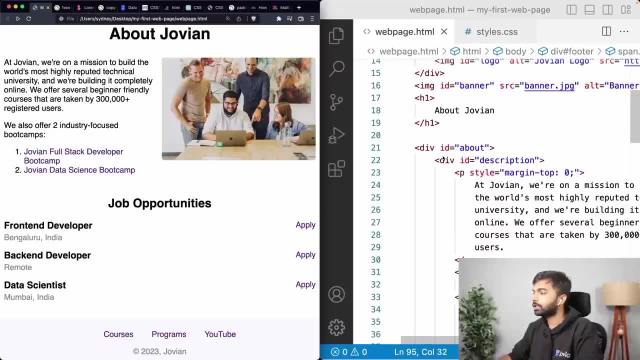 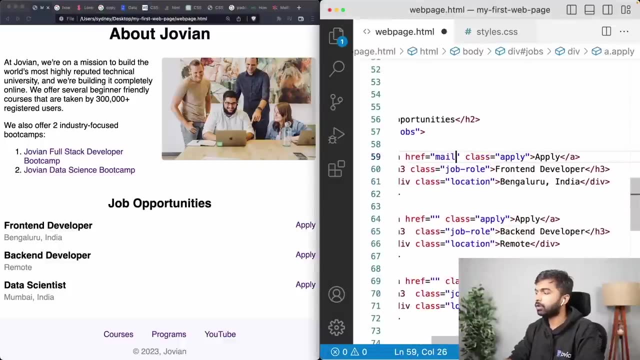 application and put in this address on the subject line. Okay, So that's a very interesting hack. So this is what we can use here for our apply, So I can go in here into apply. Where is my apply? Yeah, I can go in here and in the href I can say mail to. I can just say mail to support. 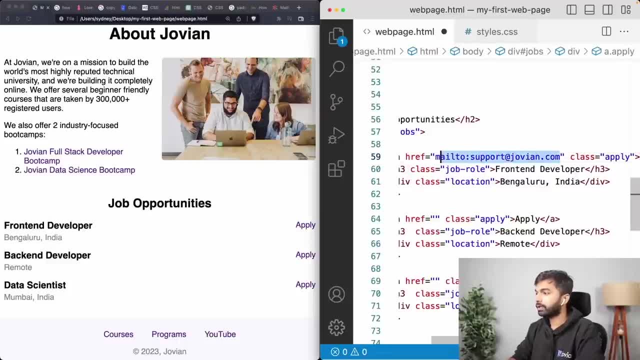 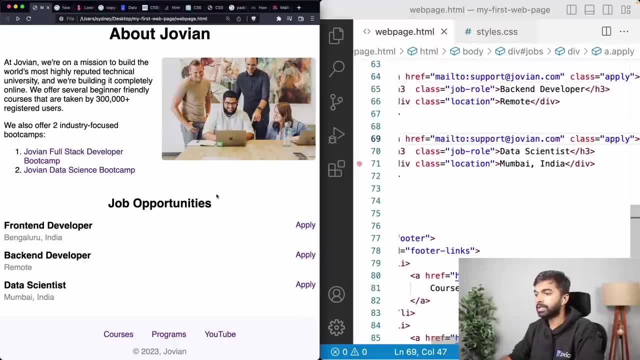 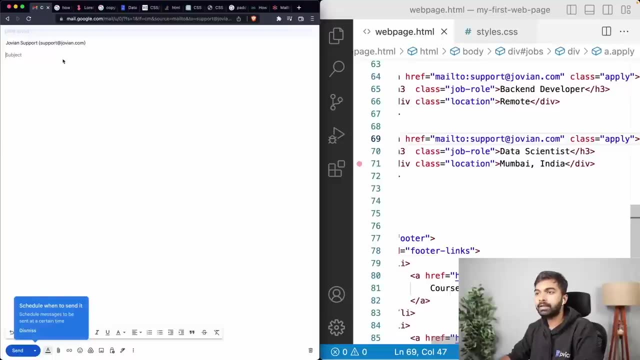 at joviancom. Okay, And let me come in here and let me say mail to support joviancom and mail to support joviancom and reload the page. Now, if I click the apply button, you can see that it opens my mail application, which is Gmail, and it is automatically filled in the address. support at 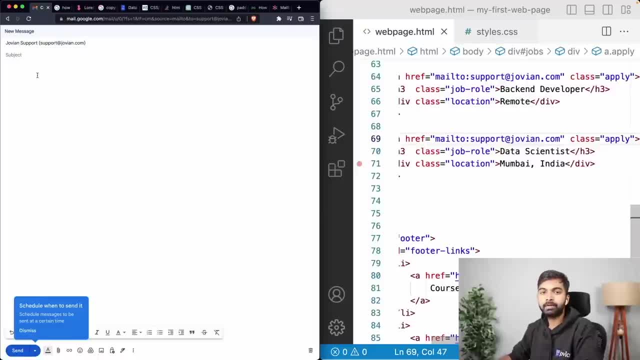 joviancom. Okay, And then here you can actually then fill out the subject and you can send an email. So essentially, what we're saying is, when the user clicks on the apply button, that is going to trigger their email client and they can just send us an email that they're interested in a particular 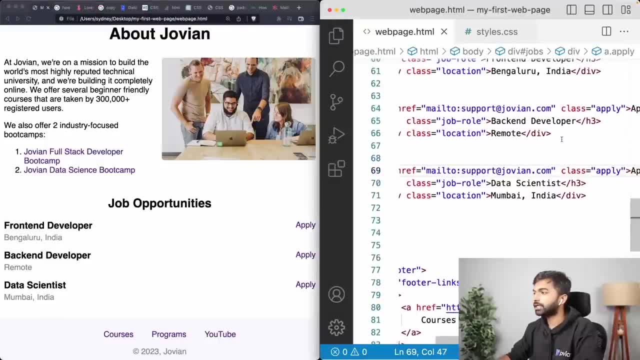 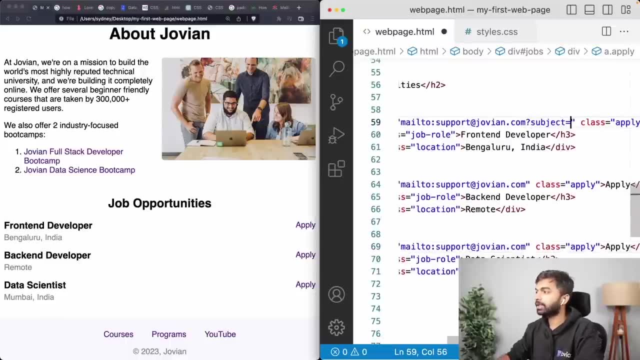 job. One thing that we can also do is we can also put in a subject here So we can say mail to and you can just say subject. you can say question mark subject after the email address equals front end and question mark subject equals back end and question mark subject. 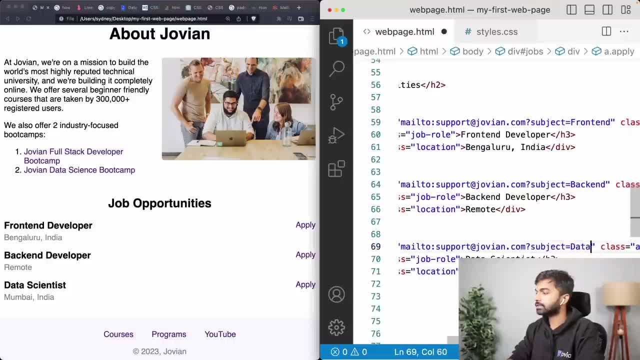 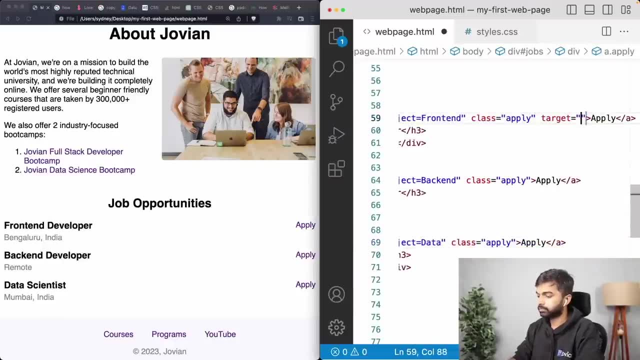 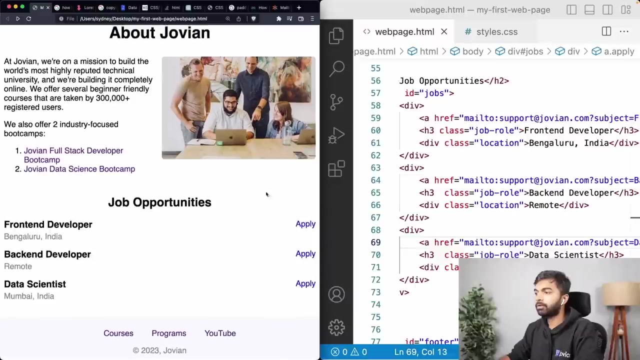 equals data scientist, or just say data. All right, And I'll also add a target underscore blank, so that it opens in a new page, Underscore blank. And let's add target equals underscore blank. and let's add target equals underscore blank. Okay, So now each of these main two links is going to have a different subject. 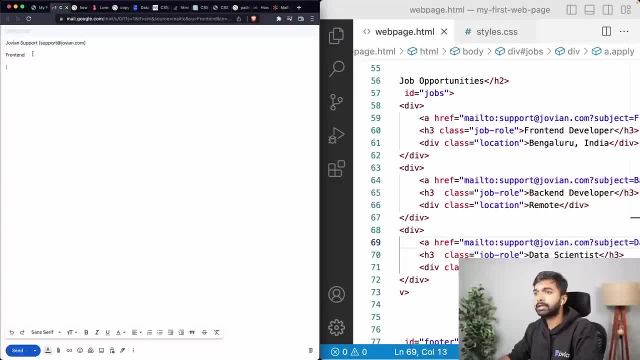 and it's going to open a new tab. you can see here that it has automatically added the subject front end and you can construct more complex subjects And in fact you can also set up some kind of a body directly as well. And similarly you can go in here and let's click on back end. 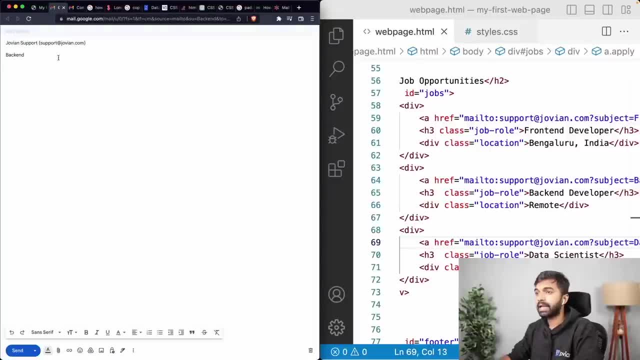 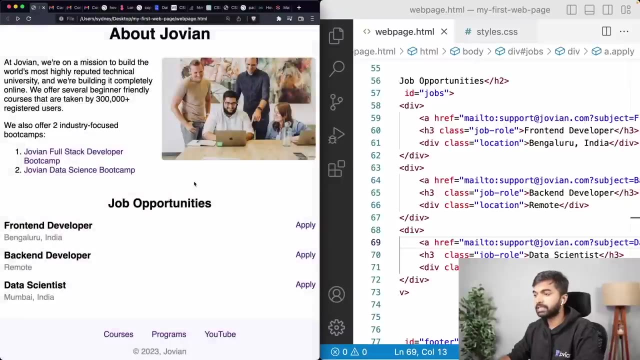 developer And it fills up the subject backend. And you can go in, click on the data scientist and it fills up the subject data. Okay, great, And then all these other links are working fine as well. I think I'm very happy with this. I'm very happy with this web page at this point. 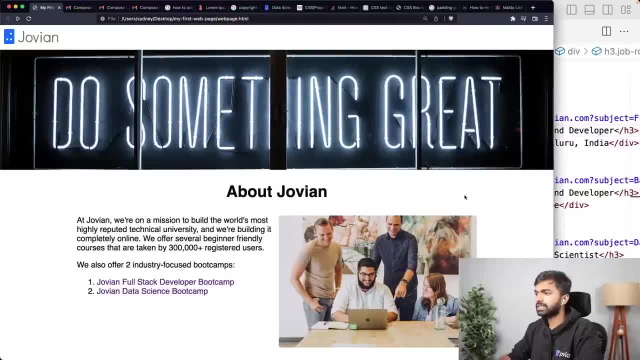 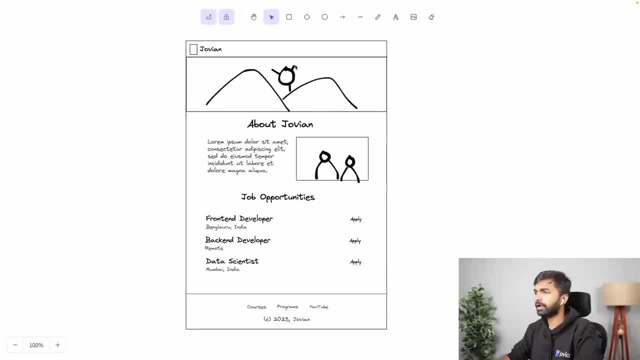 I'm just going to save it And let's see. I'm just going to reset the zoom level, Okay, so this looks good at the normal zoom level And it contains everything that I'm looking for. I have the header, I have the banner. 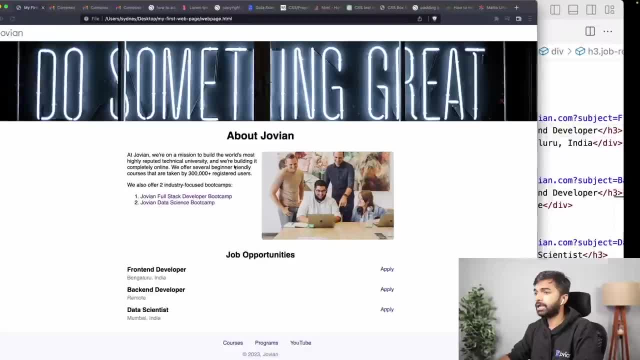 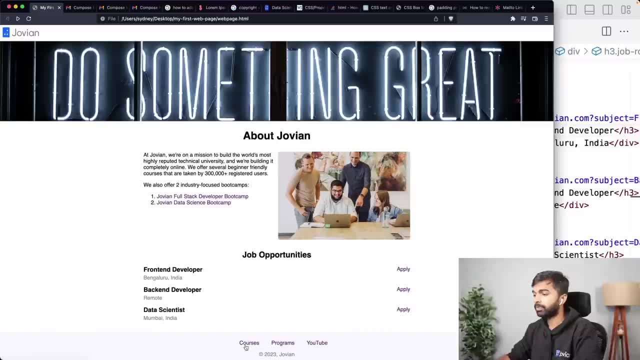 I have this section, I have some text on the left, I have something on the right- Yep, I have a couple of links here as well. I have the job opportunities And I have locations. I have this apply button, And then I have this footer, and then I have this copyright at the end as well. Great. 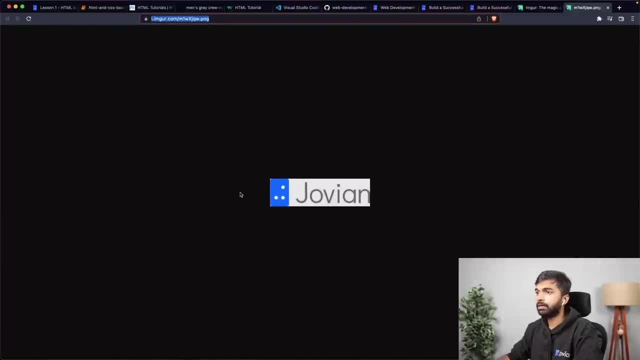 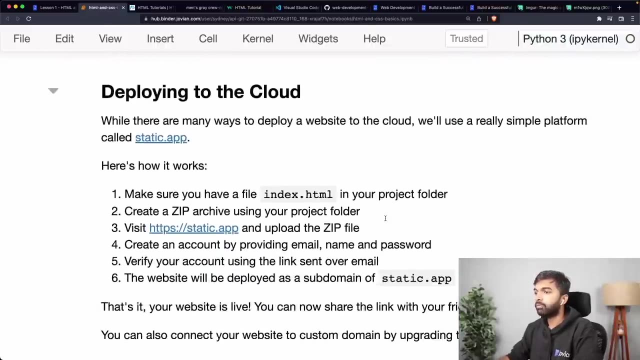 So I'm feeling very happy with this web page. Now the final step: we have completed this web page. the final step is to go ahead and deploy it. So this is what it looks like roughly, Now we can deploy this web page to the cloud. Now we're going to cover. 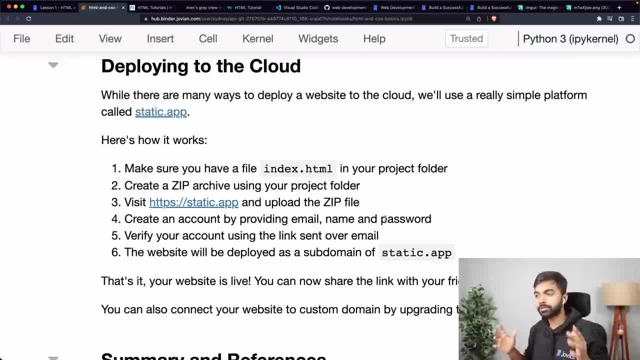 deployment extensively over the course of this program or the course of this next few lessons as well. And there are many, many ways to deploy a website to the cloud. there are hundreds of platforms, But the simplest thing is to just upload a zip file, right? Wouldn't it be nice if we could? 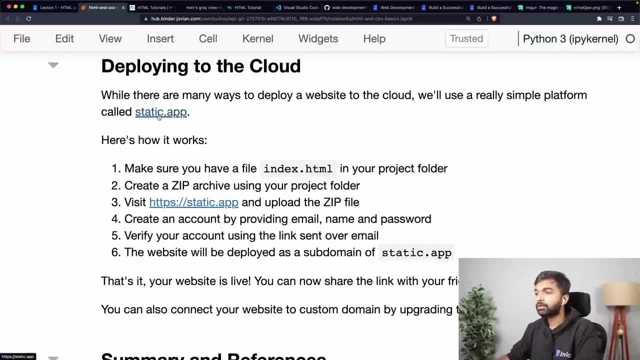 just zip up our web page and just upload it on the cloud. Well, that is what you can do using this platform called staticapp, And then, after that, you can even deploy a web page or a website to the cloud. So I'm going to go ahead and deploy a file to the cloud and upload it to the web page, And now. 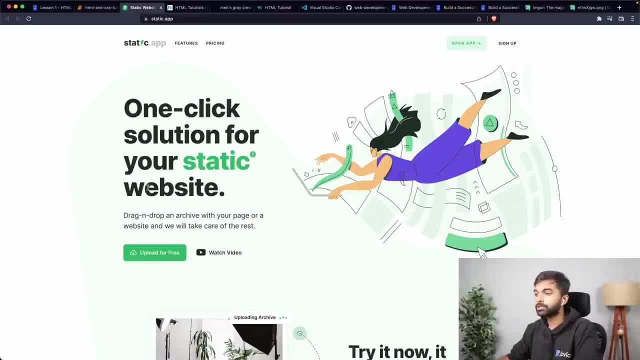 app, and there are a bunch of these platforms, but staticapp allows you to simply drag drop an archive with your page or a website in it and it will take care of the rest. okay, it'll automatically set up a website for you. now, here is what we do. first, we have to make sure 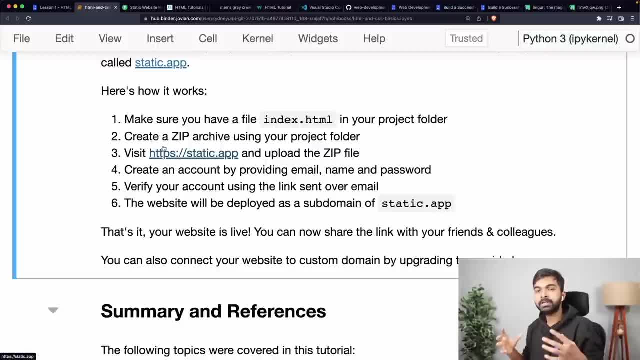 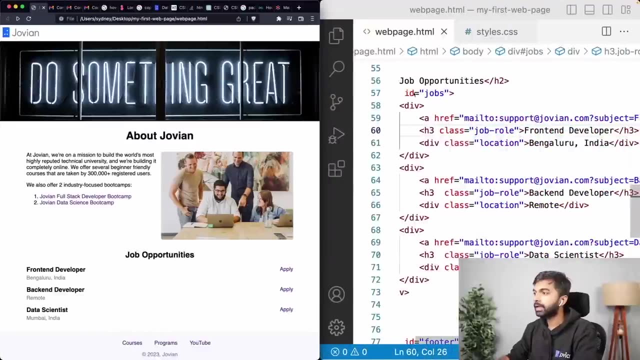 that we have an indexhtml page. so there is this convention in html that a file called indexhtml is going to be the root page of a website. okay, or the root page. so when you open joviancom, that's actually opening jovicom indexhtml. so let's go back here and let us rename web. 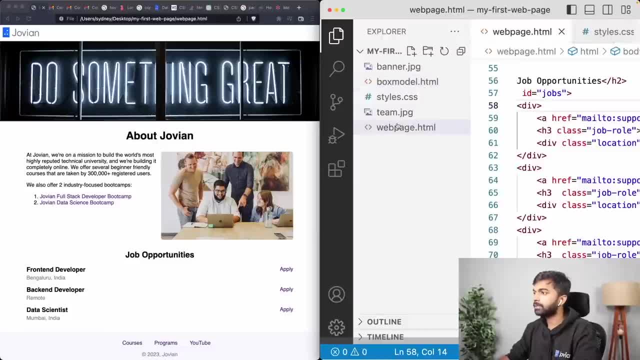 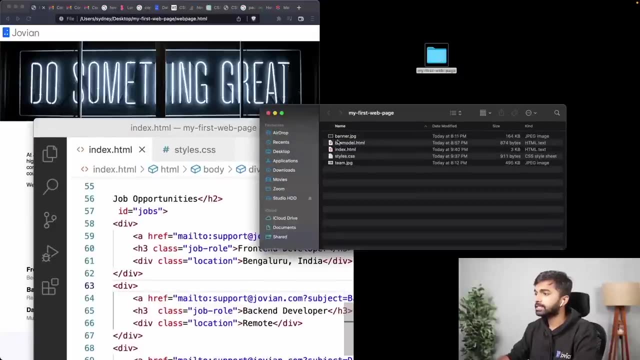 pagehtml to indexhtml, so let's rename this to indexhtml and then let us go and zip up this folder. so we have this folder over here which has a indexhtml file which is the sort of the root page or the root web page, and it has a bunch of other files and images that we 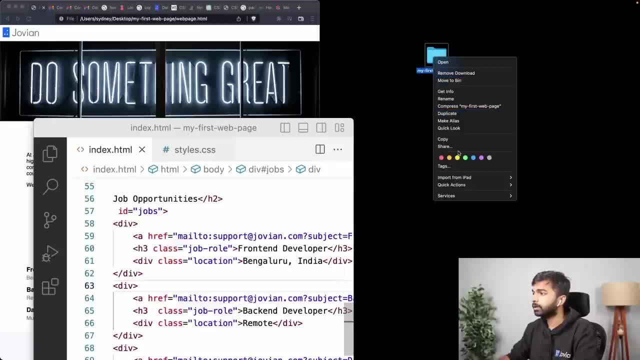 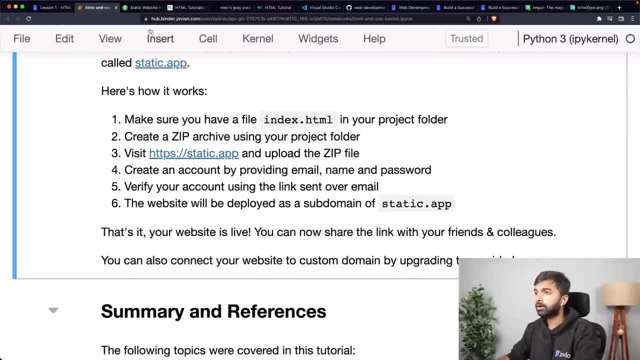 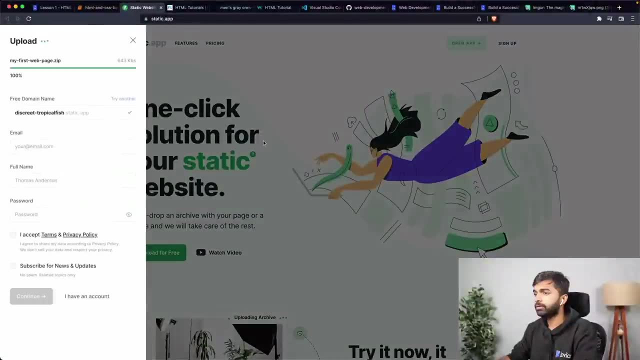 can use as well. i'm going to zip it up, so i'm going to say compress, and depending on your operating system, you may have a different way to zip things- and then on staticapp, i'm just going to click upload for free. i am then going to upload this zip file over here and that is going to then. 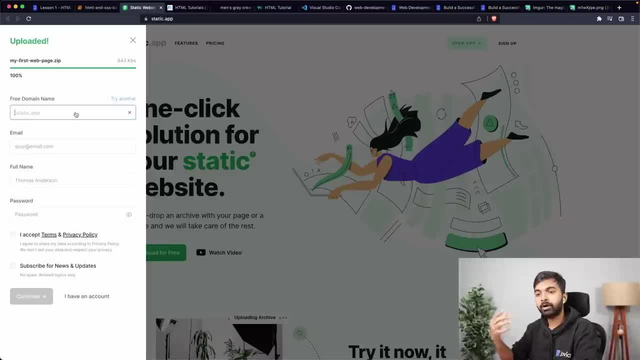 ask me to maybe pick a domain name, so it's going to be a sub domain of staticapp, so let me just put it as joviancom. i can't spell my own company name, okay, and let me just put in an email here. sydney is the account i'm using: sydney, joviancom. 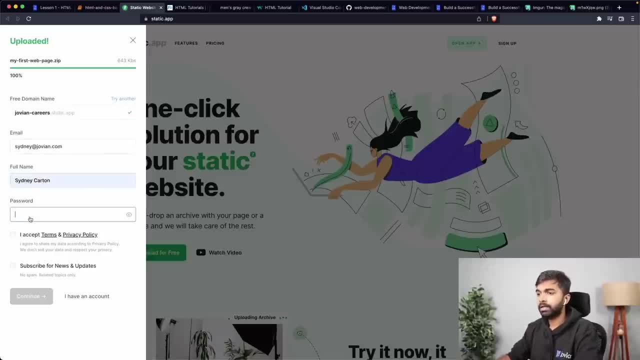 and let me put in the name here: sydney carton. okay, let me put in a password here. i'm not going to say that and let me just accept the terms of privacy and let me just say continue. okay, looks like this email has been taken. let me just provide a slightly different. 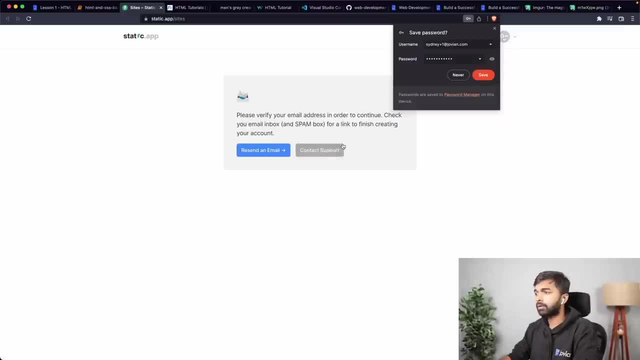 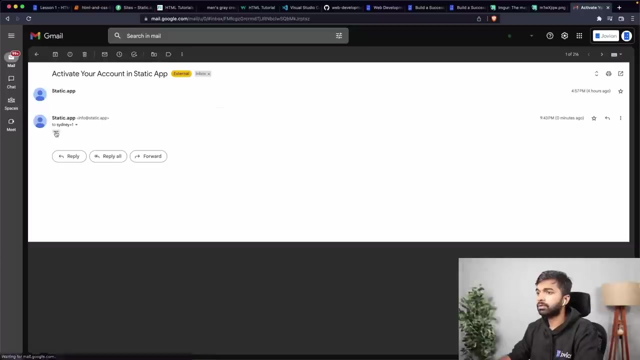 email. yeah, so now that is going to ask me to verify my email. i've uploaded the zip file already, so i'm just going to go ahead and verify the email i am going to. let's see, let's open up emailcom, and here is the account and here is the verification link. 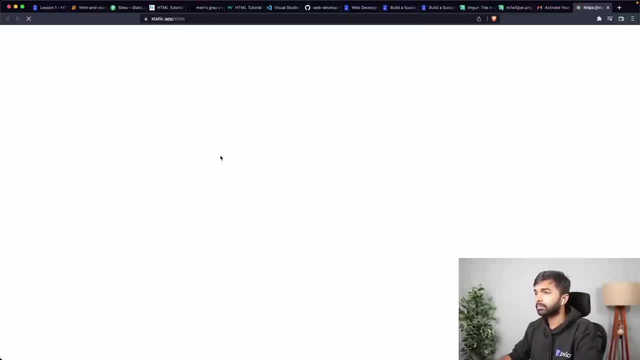 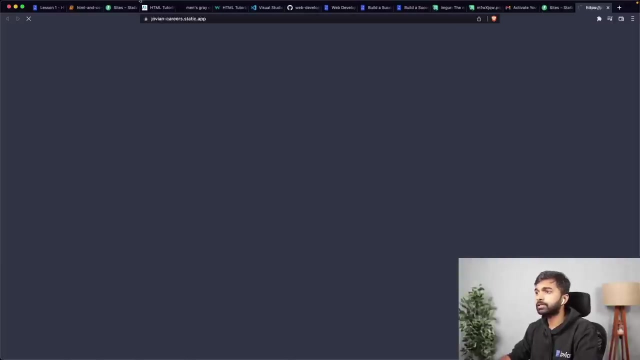 okay, my email is verified and now you can see that joviancareersstaticapp- this website- is getting deployed. okay, so let's give that a couple of minutes. looks like it is deployed, so let's maybe go and check it out. let me just click joviancareersstaticapp. 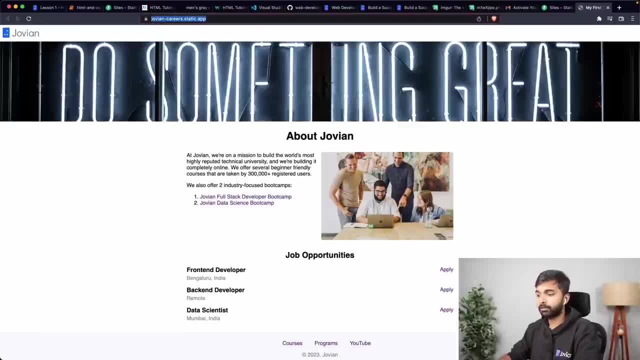 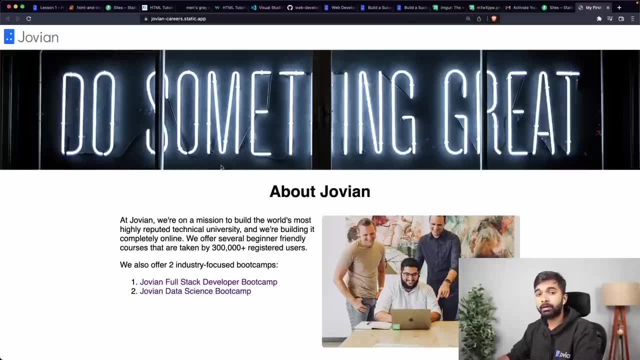 and yes, looks like this website is already deployed and in fact, you can open it up on your end as well. and because we have set up, because we have set up this page, welcome webpagehtml as indexhtml. that is why it's opening up directly, but i can also just type indexhtml and it will. 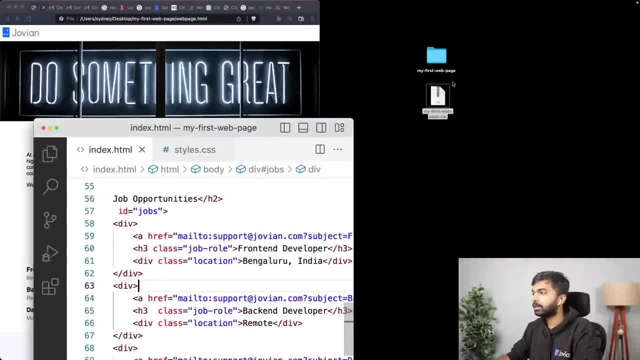 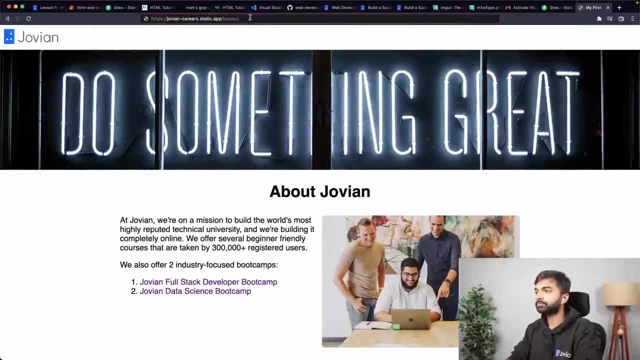 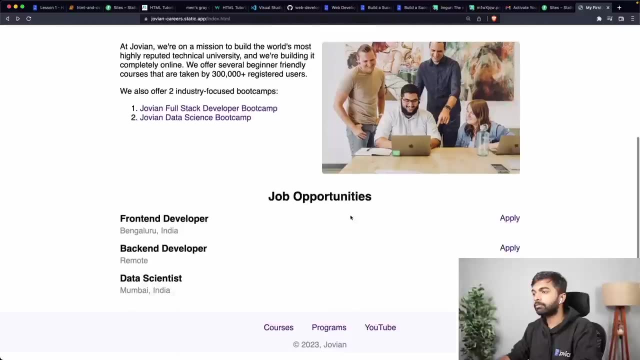 open the exact same page. okay, not only that. remember we have this other page called boxmodelhtml. well, boxmodelhtml should open up, just fine as well. there you go, boxmodelhtml. and in fact, if we had a link here from indexhtml to boxmodelhtml, then that link would work properly as well. and you can see that both these images got. 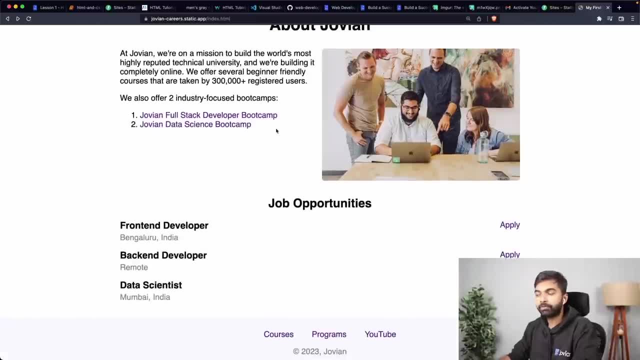 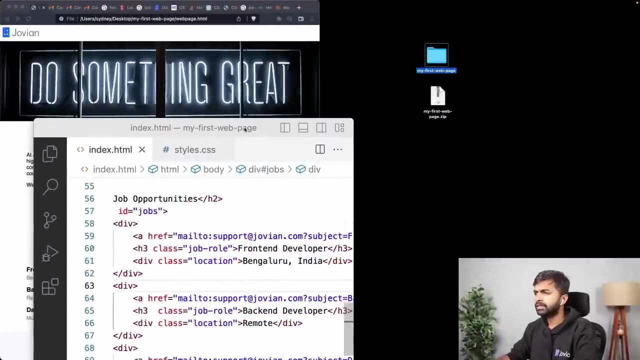 uploaded as well. so that is how you deploy a site, the. the simplest way to deploy your site is to just zip up your code and put it up online. you don't need any git aws, deployment commands, etc. it's all really simple to do, okay, and that's it. so let's take a quick summary of the whole thing. 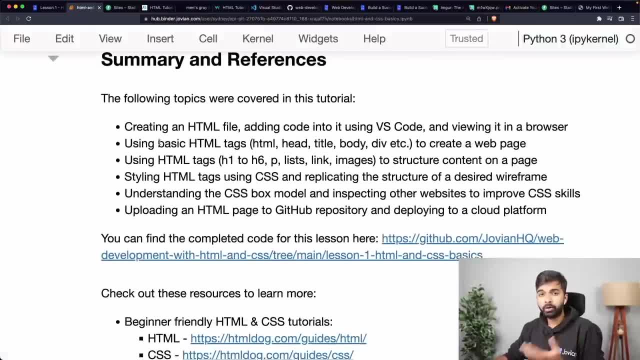 here's what we did: we created an html file on. we created a folder on our desktop, we put in our html file into it. we added some code into it using the html file, and we added some code into it and then we tried to view it in a browser. then we using some basic html tags like html head title. 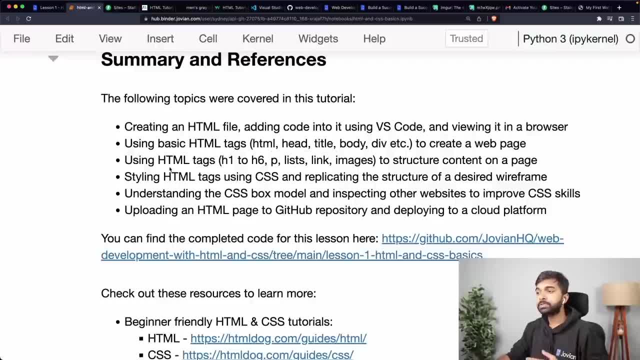 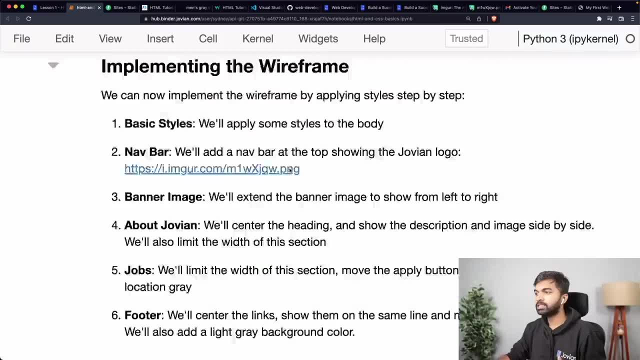 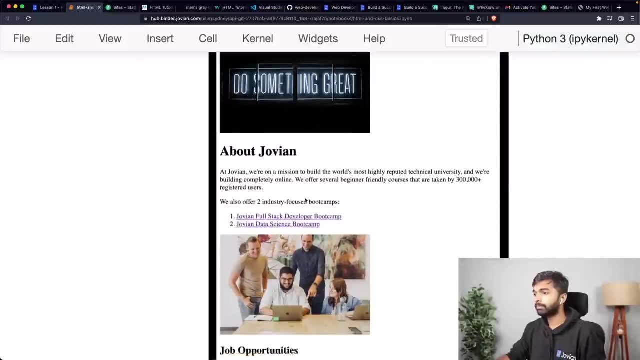 body, div, etc. we created a web page. then we use some more html tags- h1 to h6, p list links, etc. to structure content on a web page. so remember this piece. before we added any css, we just put up a bunch of content on the web page and here is what it looked like. then we learned how to apply. 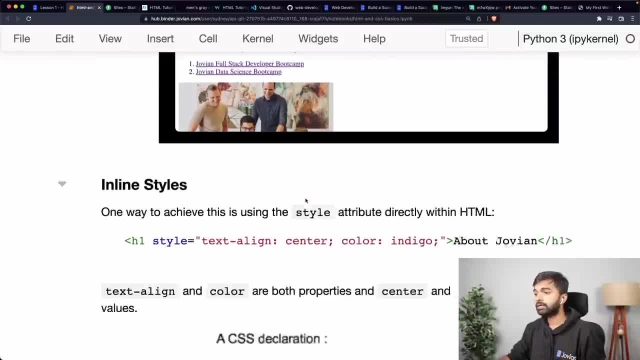 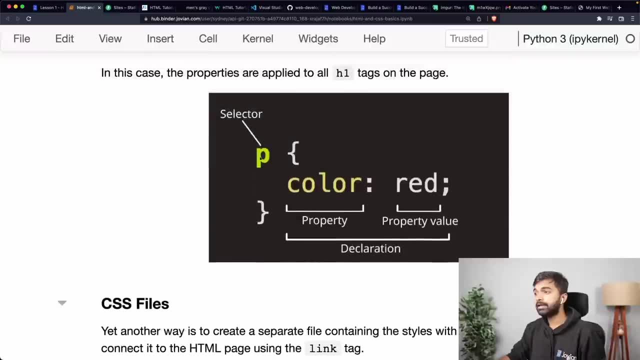 styles using css. so cascading styles using css. so cascading styles using css, so cascading styles sheets. the way we saw that. we saw that we can apply styles inline. we can apply styles using the style tag, we can apply styles using CSS files. and the key idea: 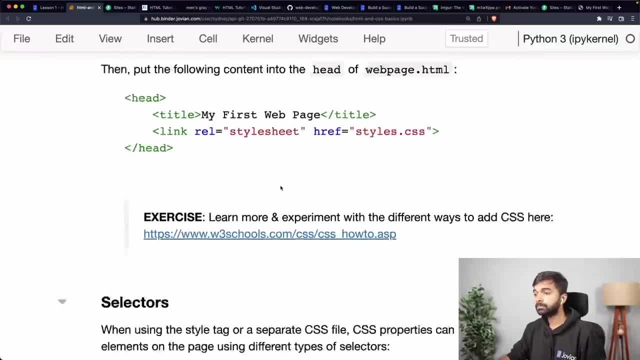 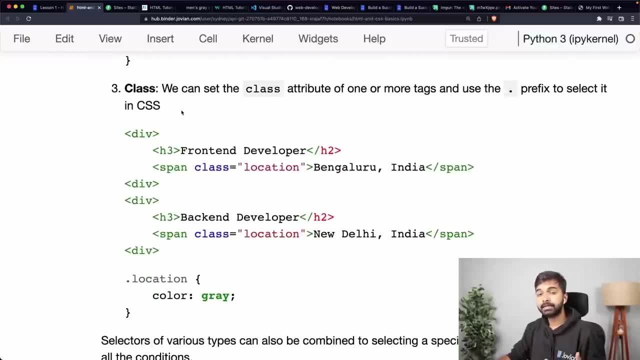 is you have a selector and then you have a property and a value. Then we looked at the different kinds of selectors. We have tag selectors, we have ID based selectors and we have class selectors. Then we learned the CSS box model, which is how you have content and then around. 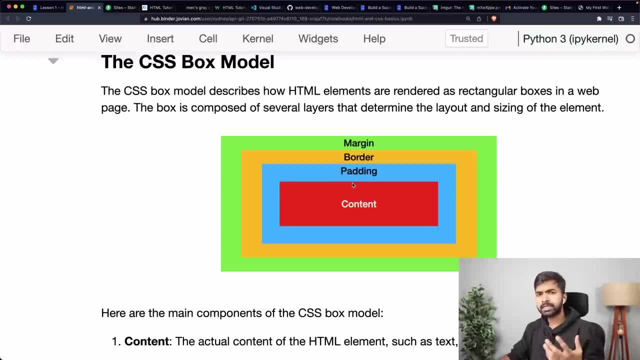 the content. you can add padding and the padding is also shares the same background, And then the padding is inside the border. The border is something that you can set width for and then outside your margin, and margins can overlap for side-by-side elements. 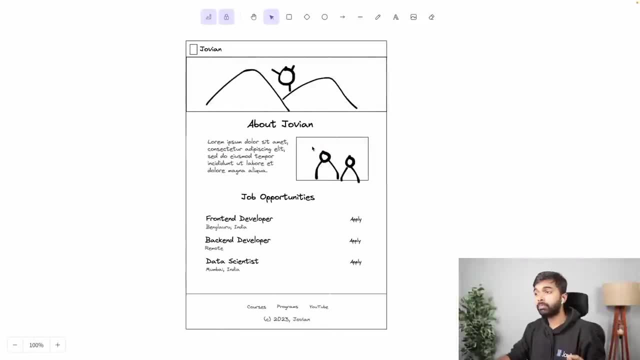 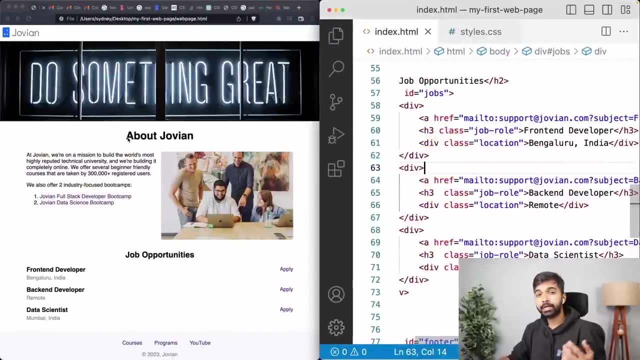 And then we, of course, we implemented a wireframe using Excaliburcom and we then tried to replicate this wireframe within CSS you by adding a bunch of CSS properties starting from the top. So we picked section by section. 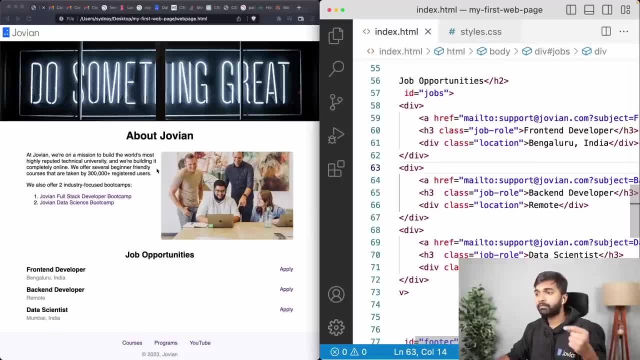 We added an app bar, We added a logo in it, We fixed the banner, We fixed the section about Jovian, Then we went Into job opportunities And then we added a footer right. So that's what we did. 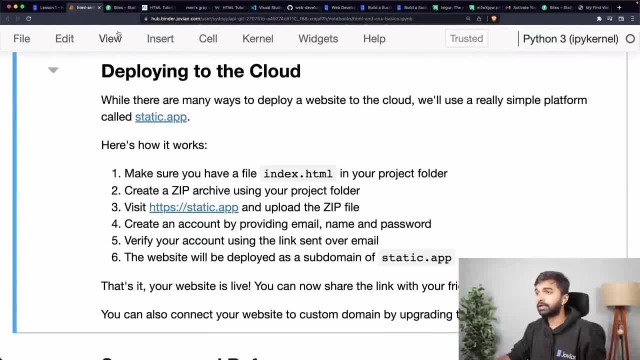 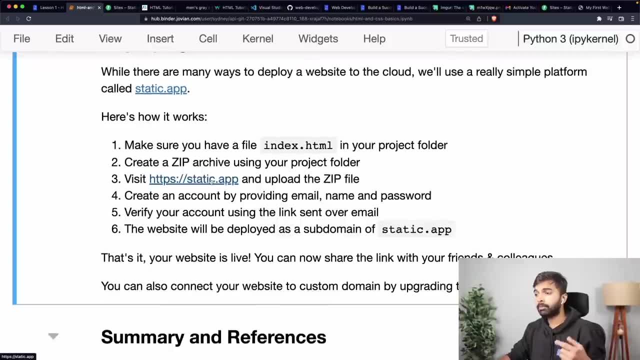 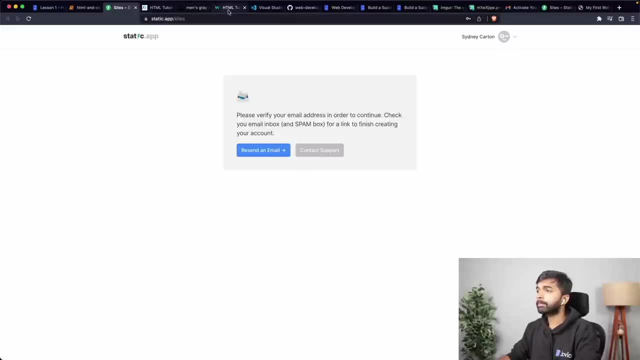 And finally, we just deployed our website to the cloud using staticapp. We just went to staticapp, created a zip file, renamed our main page to indexhtml and uploaded that zip file, verified our account and it is deployed as a. um yeah, 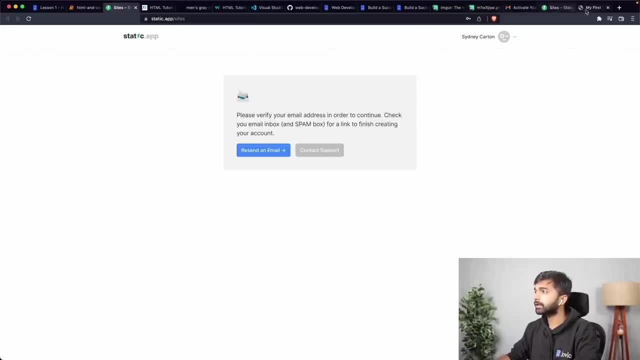 So it is deployed. Where is it? Yeah, it is deployed as a sub domain of staticapp, But within staticapp itself you can also go into settings and actually configure a custom domain, So you can actually put this on joviancareerscom or something like that. 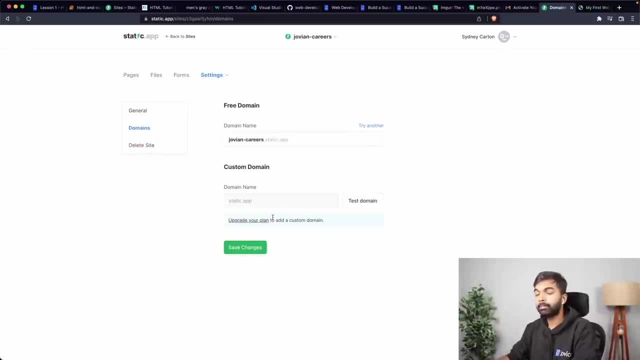 You can go in. you'll have to upgrade your plan, You'll have to pay And you can set up a custom domain. You can just set up a domain like joviancareerscom and you can set up some DNS settings and make sure that that is where your webpage shows up. 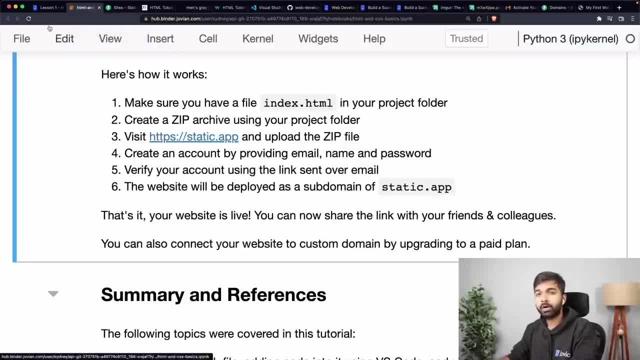 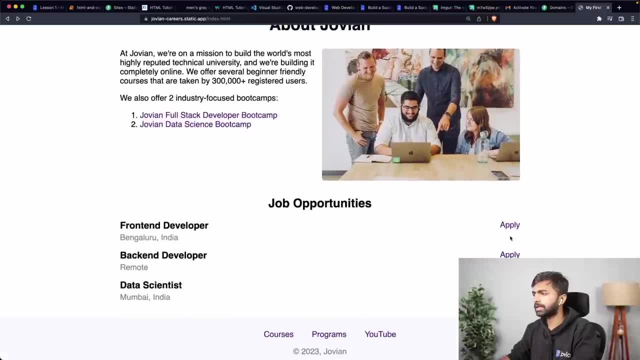 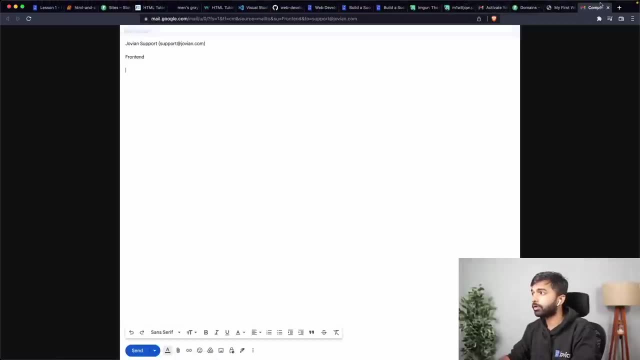 So that's not bad for a first lesson. We probably spend about two hours- two hours, 15 minutes if we exclude the breaks- and we were able to build a Pretty good functional website. and clicking on this website, the actual functionality is also present, because you can click apply and you can actually go ahead and send out an email to the Jovian team to apply for a job. 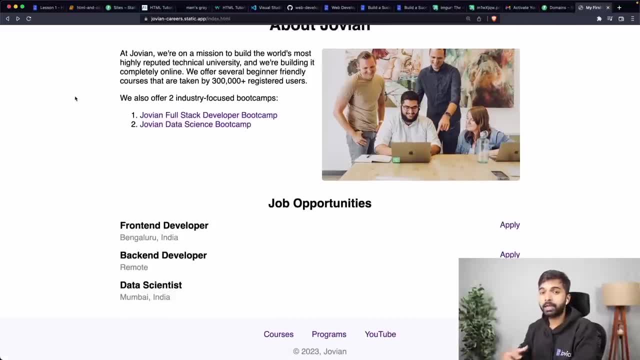 So that's how simple HTML and CSS really is, Once you can become familiar with just the most basic parts. And, of course, there's a lot more to it. There are tables, there are forms that have various CSS properties- flex box, et cetera. 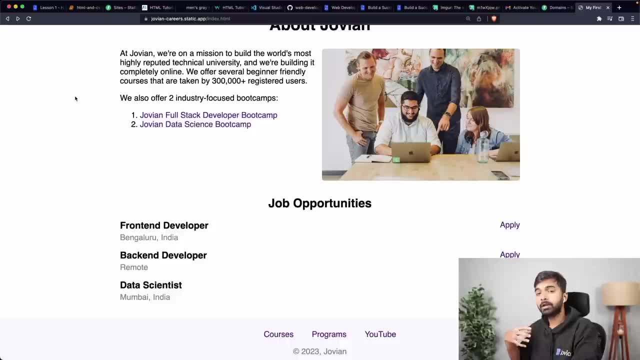 But what I want you to take away here is that you should try to first figure out what do you want to build, And try to build it using what you already know, and then just try to learn, as you go along, the things that you don't already know. 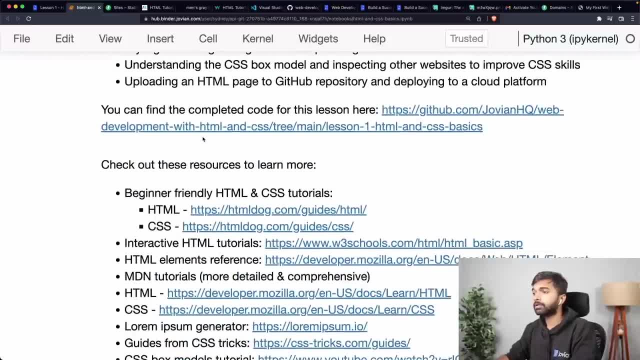 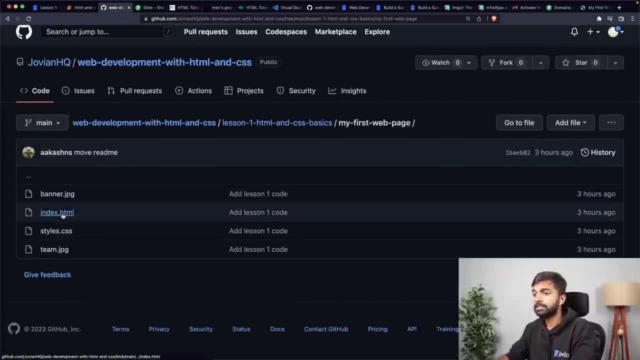 Okay, And here are some references that you can check out. You can find the completed code for this lesson. It may be slightly different because we've done this live. You can find the completed code for this lesson here. You have this indexhtml over here, but that's great. 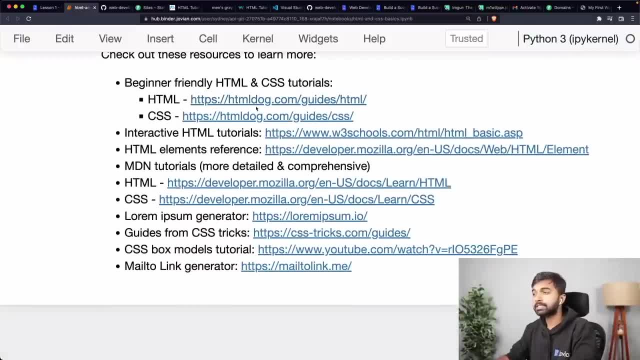 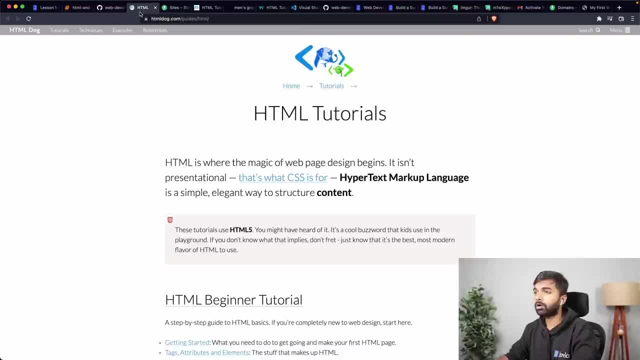 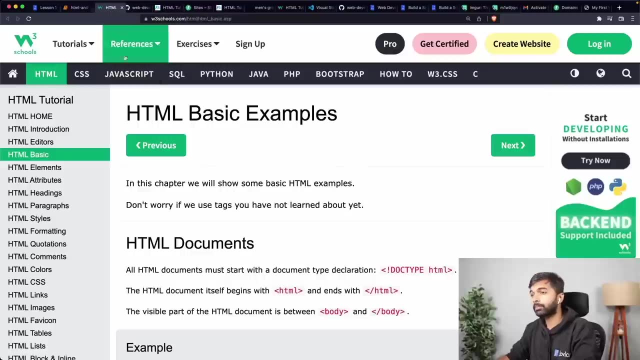 And then you have maybe some beginner friendly HTML and CSS tutorials. in case you want to look at other tutorials as well, Okay, After practicing this, you can go and check that out. So htmldogcom is something that I found very simple to follow along with, but you want some. if you want some interactive HTML tutorials, you can go to w3schoolscom. 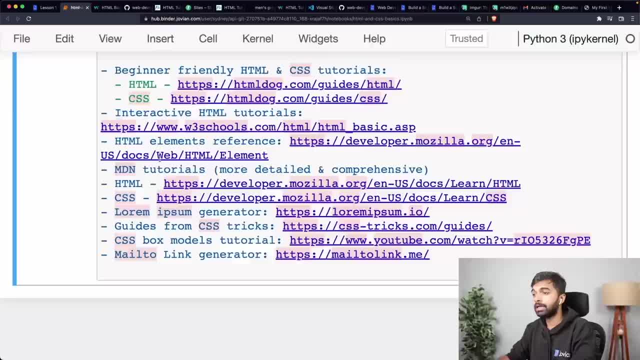 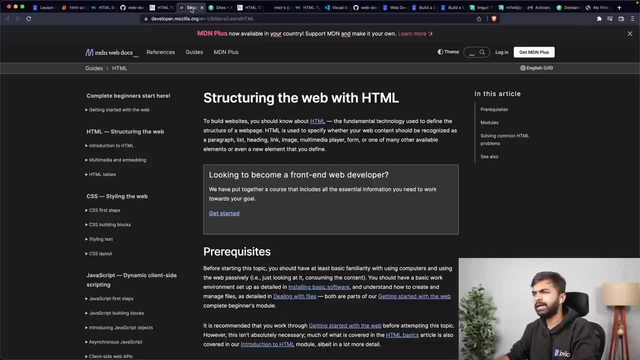 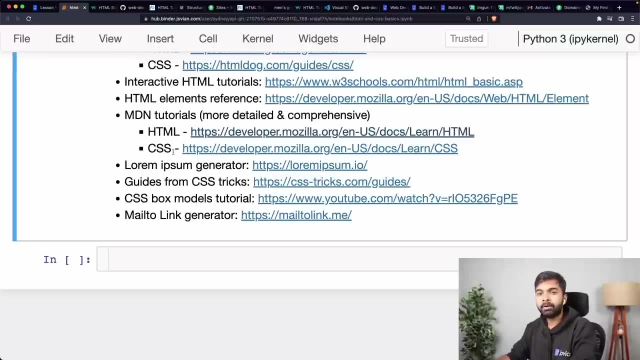 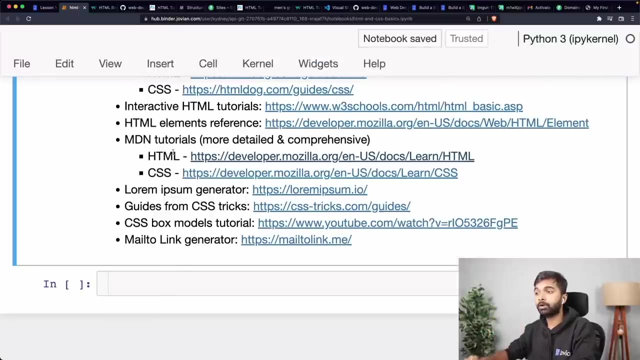 And if you want more detailed and comprehensive tutorials, check out MDN or Mozilla developer network. You can check that out as well. They have fairly detailed tutorials and a lot of explanation as well. So Take your. Depending on how new you are, depending on how comfortable you feel after practicing this lesson, after watching this lesson and practicing it, writing out all the code by hand, you can pick whichever other tutorial you want to take. 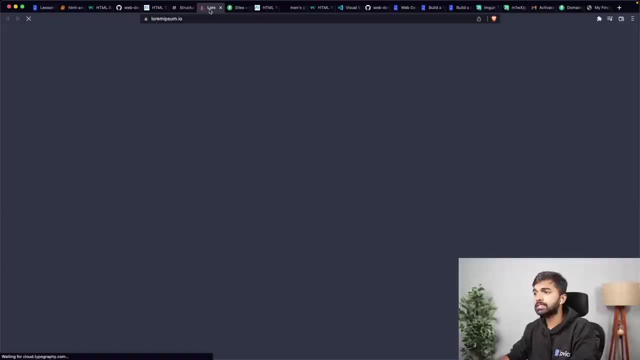 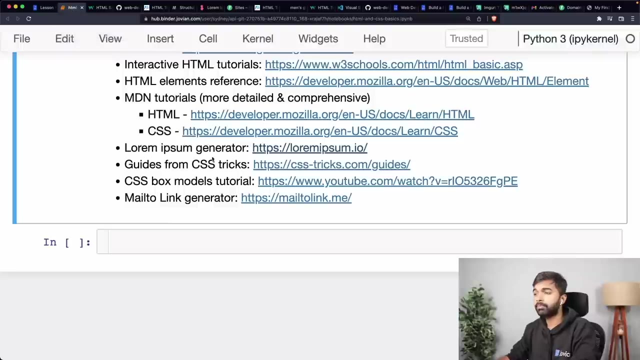 And some of the other things you can look at is the lorem ipsumio. This is the X generator that we normally use, So that's something that you can use to generate texts When you want to fill a page. if you want to learn about the CSS- CSS box model, you can check out this YouTube tutorial. 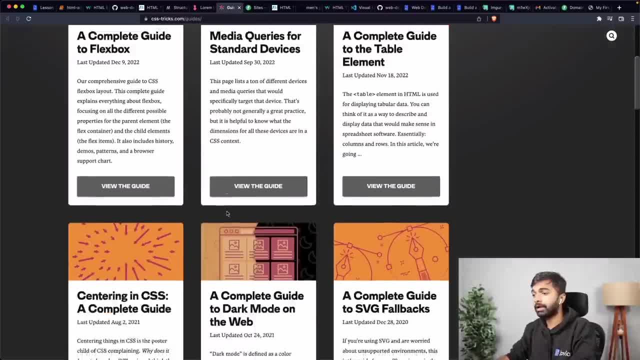 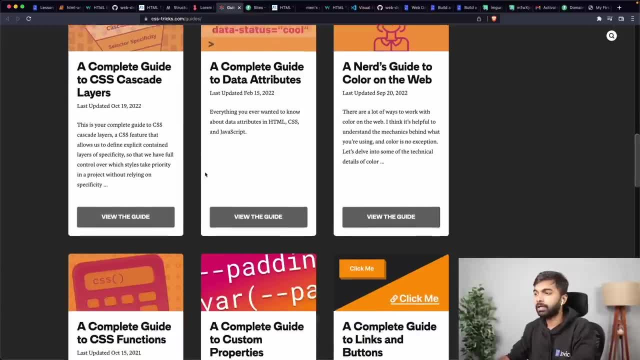 There is this website called css-trickscom. This has a lot of great guides on various topics in CSS. Don't recommend doing all these guides, but whenever you're working on a particular topic, if you need to maybe get help with a particular topic in CSS, you can check it out. 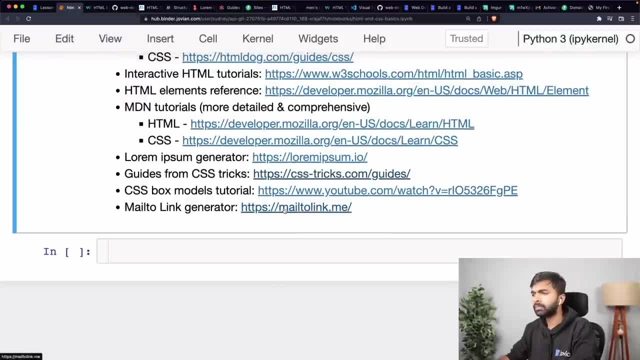 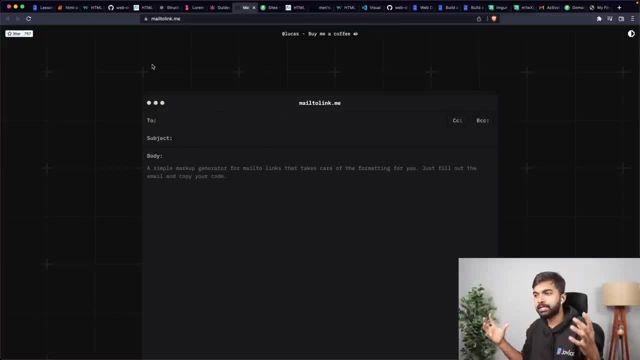 And normally you can just search online and you'll find something good enough. And then if you want to create more advanced mail to links, so you can use this mail to linkme and you can craft maybe a very interesting mail to link which can have a two line, a subject line, a body. 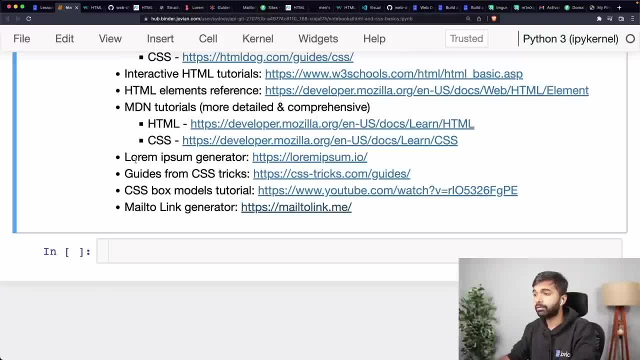 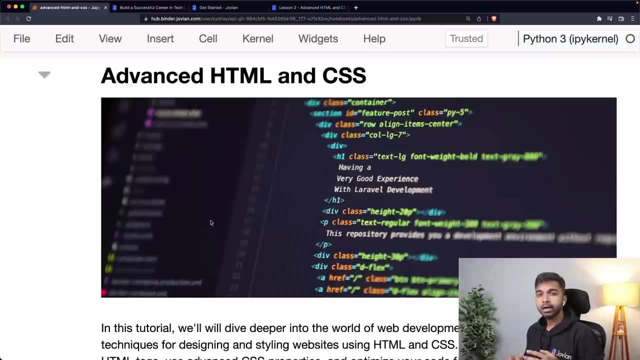 And a bunch of other things as well. You can add CC, BCC, all of that too. So the last time we looked at the very basics of HTML and CSS and we did that by working on a problem statement where we built a simple jobs careers website for Jovian. 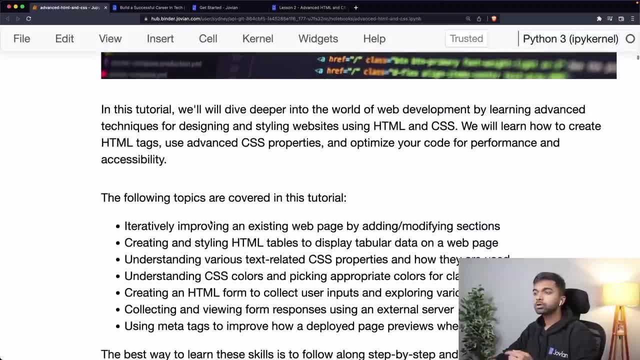 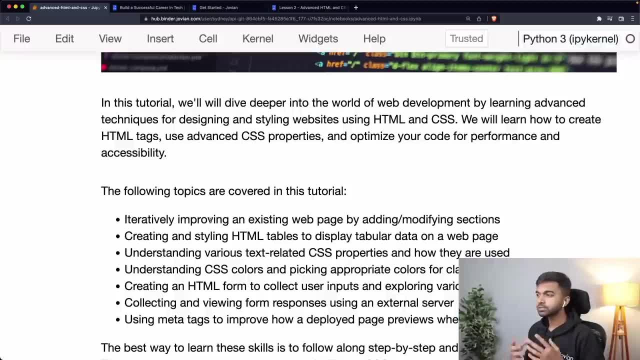 So today we are going to continue building on that. in this tutorial, we will dive deeper into the world of web development and we will learn some advanced techniques for designing and styling websites using HTML and CSS. We will learn how to create HTML tags of various types. 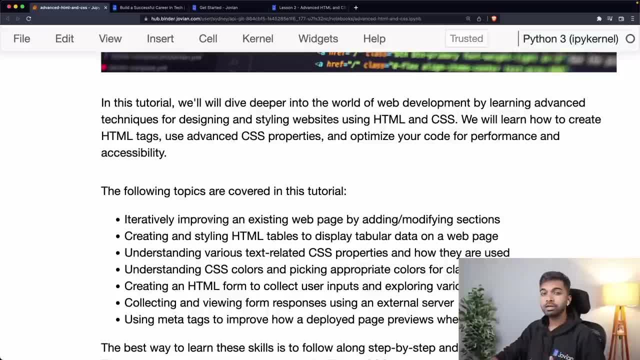 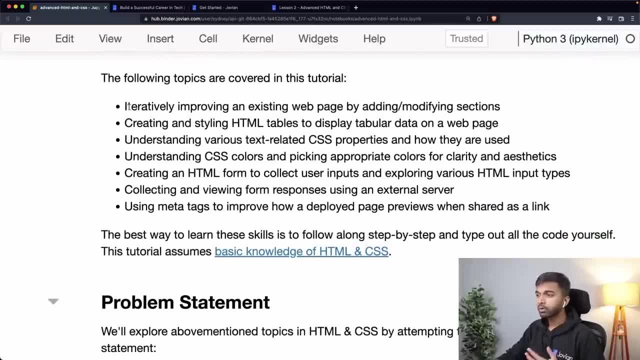 We will learn how to use some advanced CSS properties and we'll also learn how to optimize your code a little bit for performance and accessibility. So here is what we're going to cover today. We're going to iteratively improve the existing webpage. 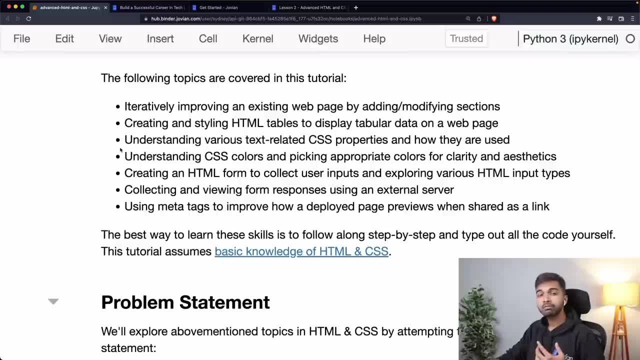 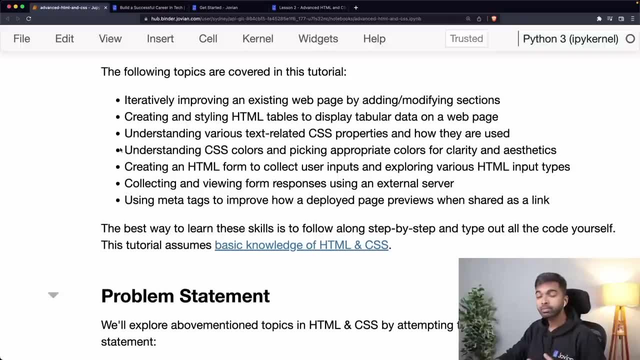 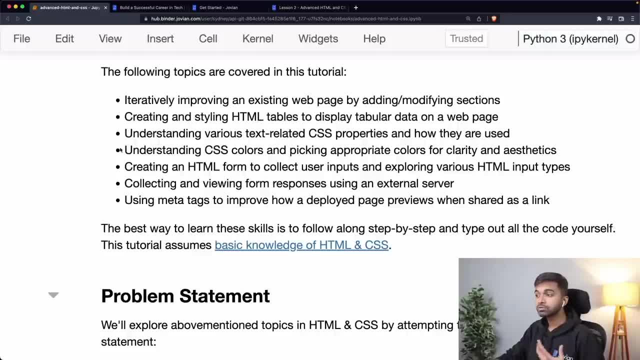 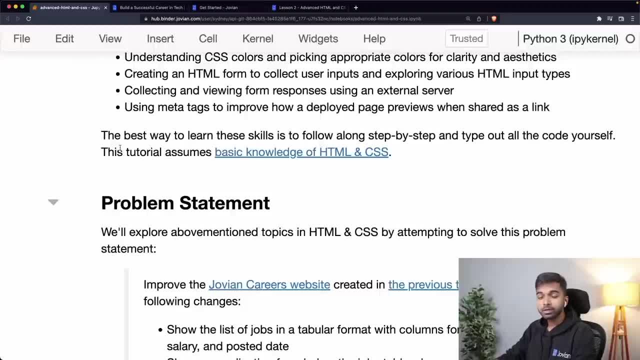 Let's get into it. And the best way to follow, the best way to learn these skills is to follow along step by step. You don't have to do that if you're watching live, but as you're watching the video, just pause at various places and try to write out all the code yourself. 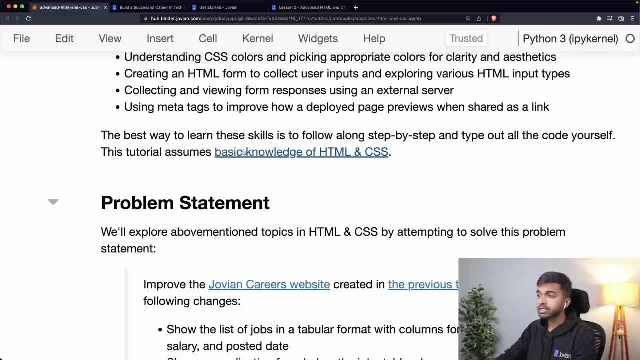 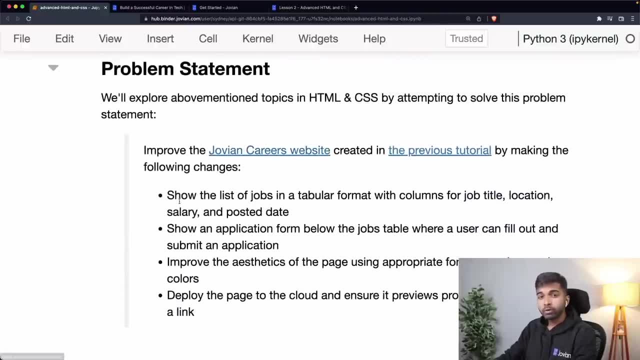 That is how you learn this quickly And, of course, we are assuming some basic knowledge of HTML and CSS here from the previous lesson, So we'll explore these topics by attempting to solve this problem statement. We will try and improve the Jovian careers website that was created in the previous tutorial. 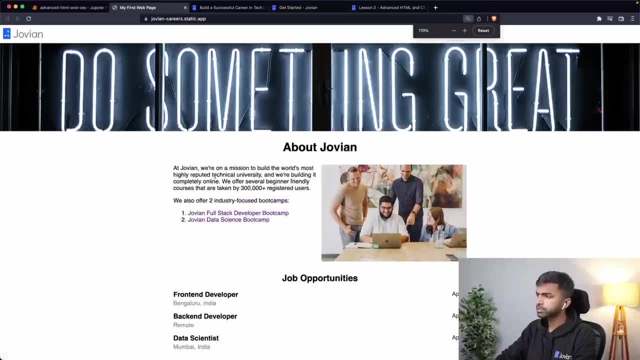 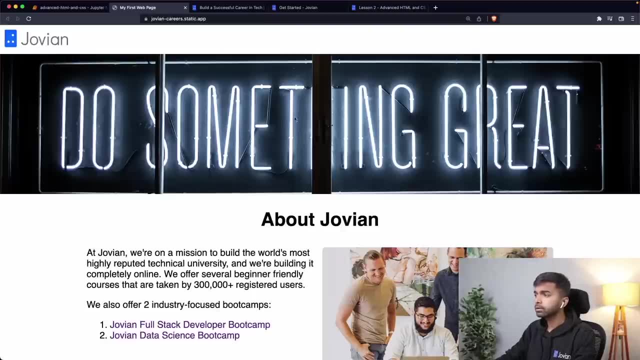 So here is what the Jovian careers website looked like. Let me zoom in here so that you can see it easily. So we have a nav bar here with the Jovian logo. We have a banner image here. It says: do something great. 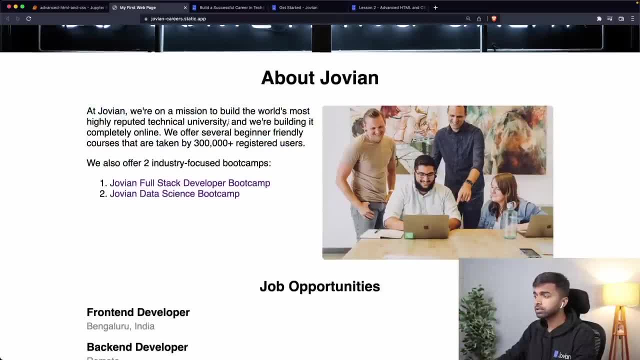 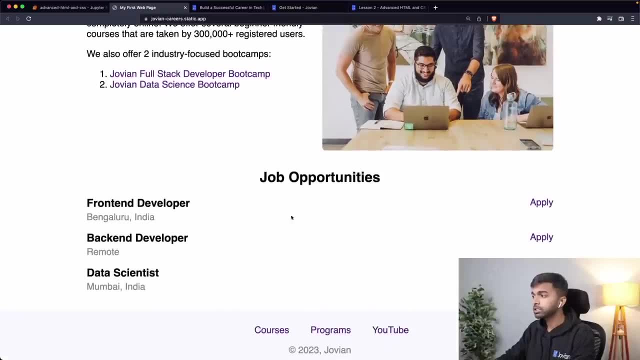 Let me have an about Jovian section, And then we have some information about Jovian. We also have an image. Ideally this should be the Jovian team, but this is just to indicate something about the team And we have information about job opportunities and you can click apply and an email will get triggered. 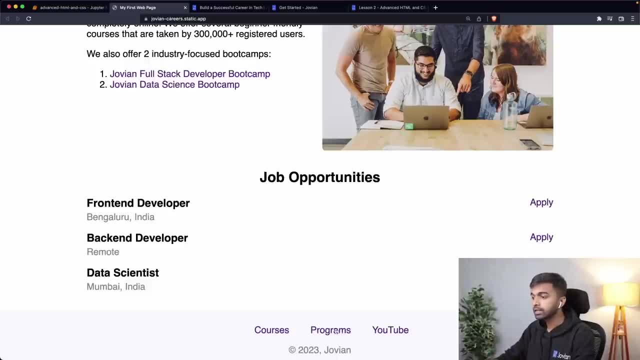 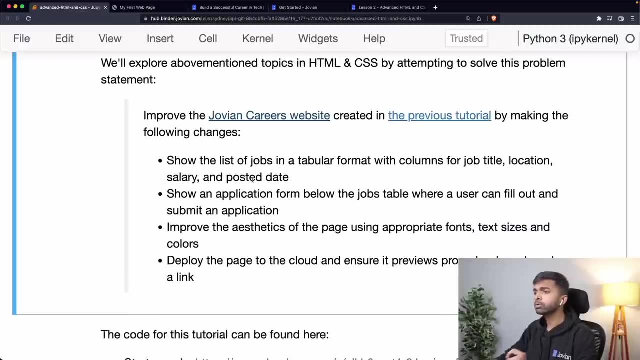 You'll be able to send out an email applying to these jobs, And then there are some links in the footer as well for courses, programs and YouTube. So this is what we built the last time, And we are going to improve upon this by making the following changes. 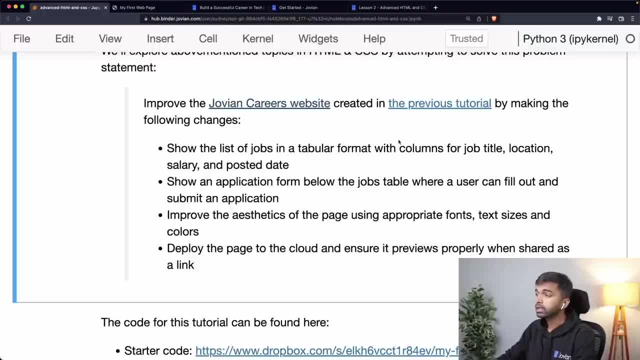 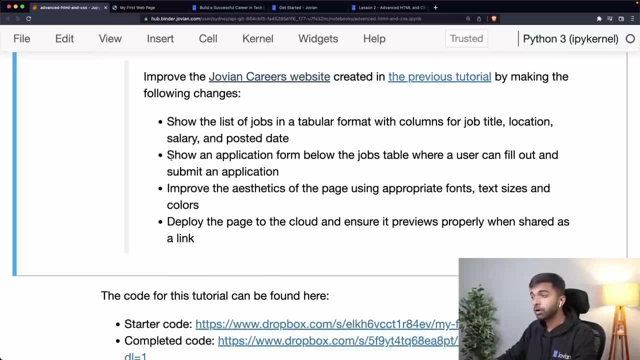 We are going to show The list of jobs in tabular format, with separate columns for the job title, location, salary and the job posted date. We are also going to show an application form below the jobs table where a user can fill out and submit an application. 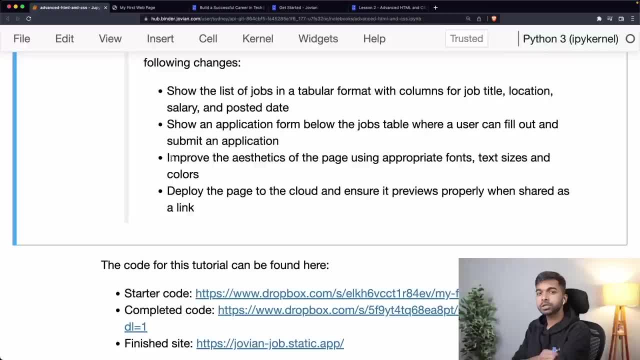 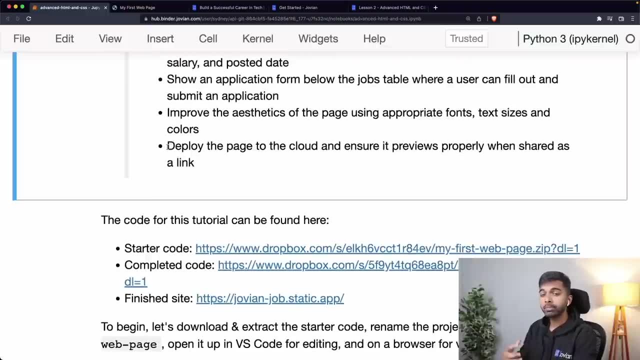 Then we are also going to improve the aesthetics of the page, Bring it closer to the Jovian brand using the appropriate fonts, text sizes and colors. Then we're going to deploy the page to the cloud and ensure that it previews properly when it is shared as a link. 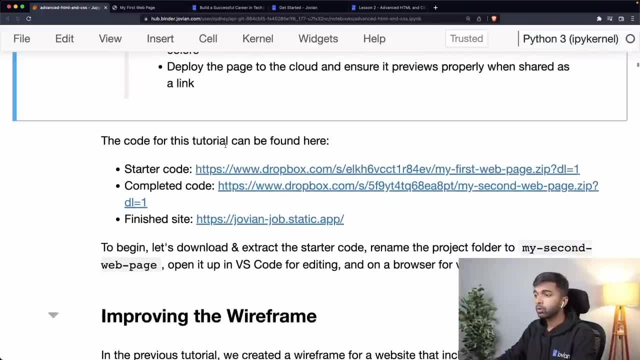 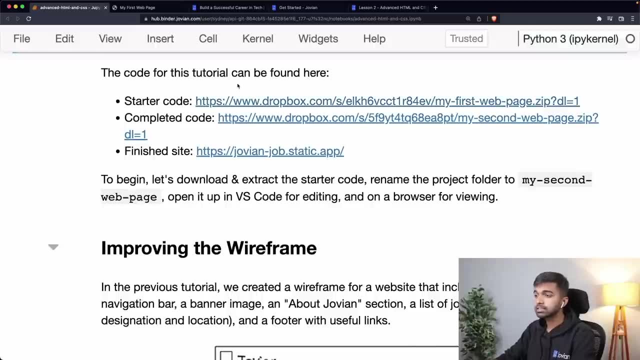 So this is what we're going to work on today. Now the code for this tutorial can be found here, So the starter code, which is the finished website from the last tutorial, is available at this link. The completed code for today's tutorial will be available at this link. 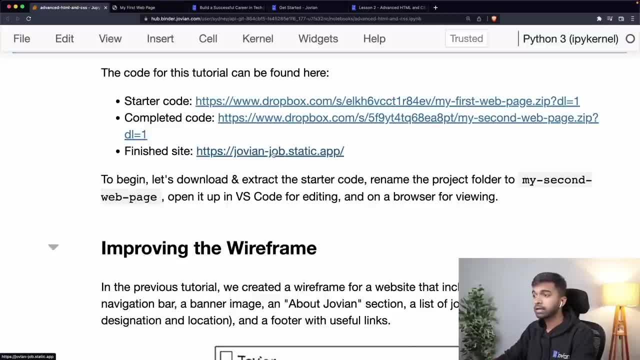 And, finally, the finished site that we are going to create today will be available at this link. So check these out in case you have, in case you face issues at any point. So let's just take the starter code and we're going to download and extract the starter code. 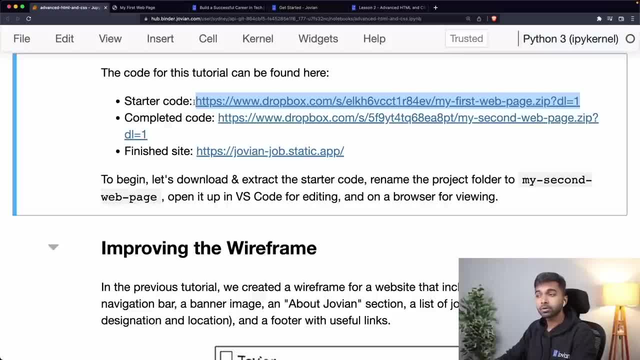 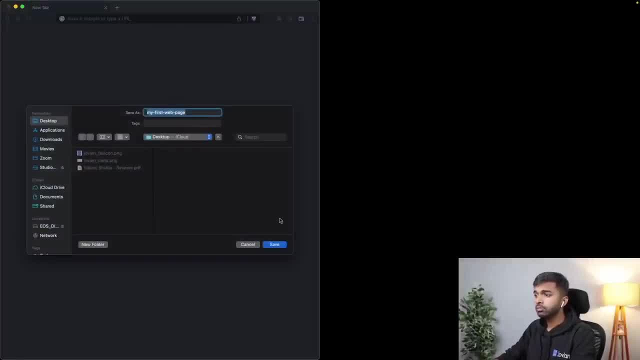 First, And then we're going to open it up in visual studio code. So let's open up this link. This contains the starter code and I'm just going to save it on my desktop. It's going to be saved with the name. 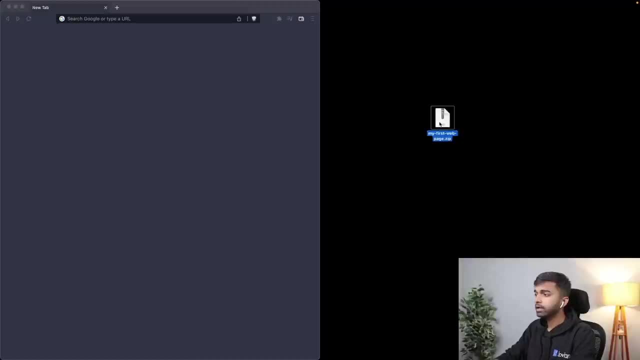 My first web page, dot zip. You can see that I have a zip file here. I'm just going to open up the zip file, So extract it. And now I no longer need this original zip file, So I'm going to delete it. 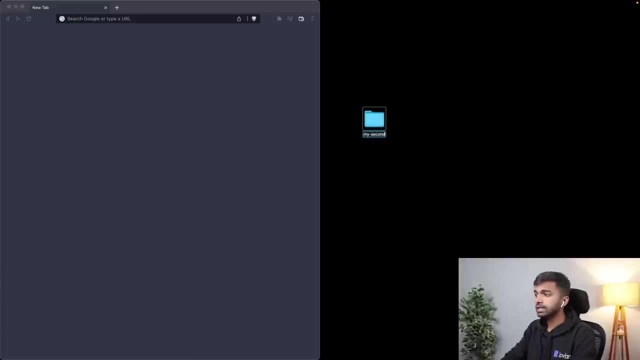 Then I am going to rename this. So I'm going to rename this to my second web page, Since this is our second web page. So you can see here I've renamed it to my second web page. Now I want to open this up in visual studio code. 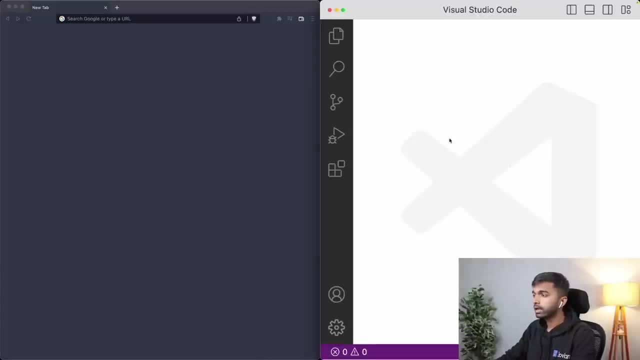 So let me open VS code or visual studio code, And I have visual studio code. I've installed it already. in case you don't know, I don't have it installed, Just go online, search for visual studio code and install it. And now I'm going to go into the file menu and I'm going to select open folder. 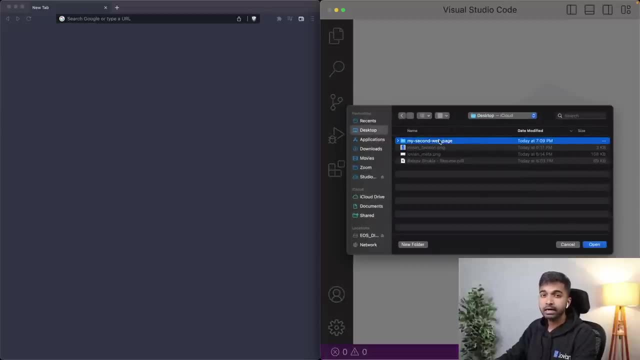 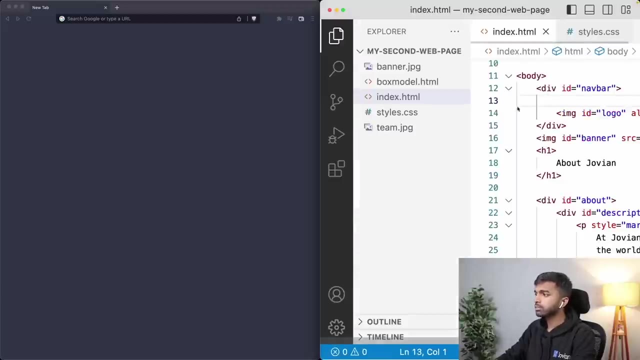 And now I'm going to just select the folder- My second web page That I have just downloaded- and let's open it up. and here you go. Now we have this HTML file, Now we have a CSS file, and we have a bunch of other files as well from last time. 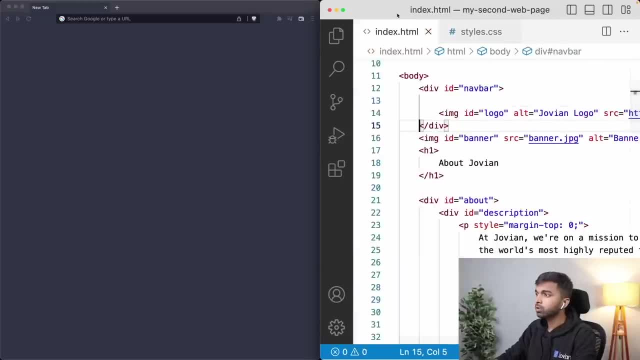 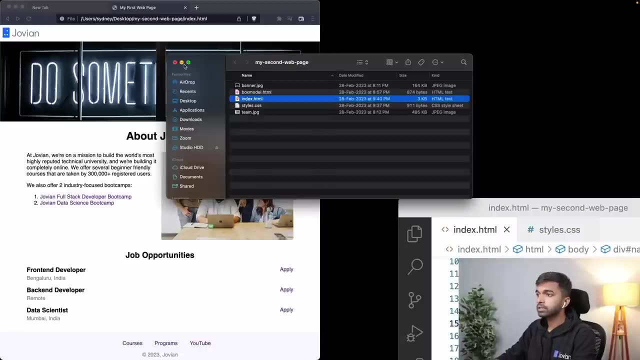 So this is all the starter code that we have, And let me also open up the web page in the browser. So I'm just going to open it up in the browser here as well, So that we have it open both for editing and for previewing. 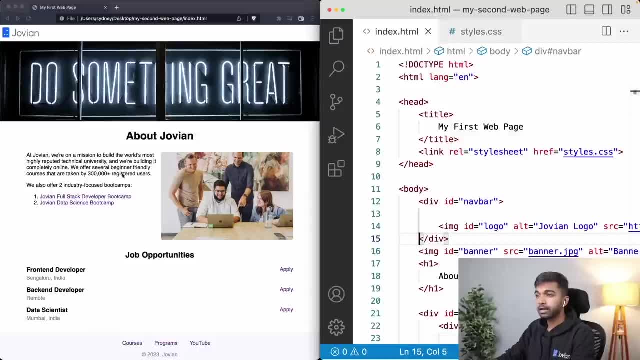 So now we have A file- indexhtml- here, and that file contains all the content for this page. Let's quickly review what this file contains so that we, when we start modifying it, we'll know exactly what to do. Now, of course, we have this head tag here, which sets the title of the page. 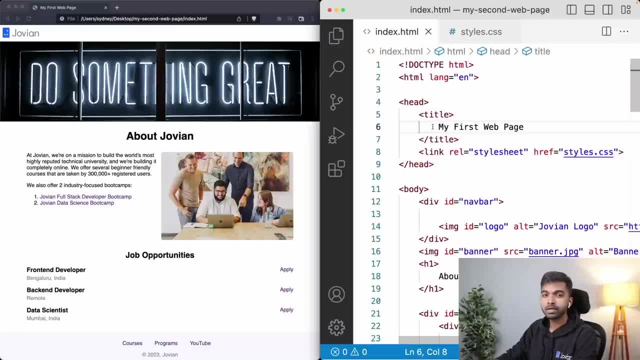 Notice that we didn't actually set a proper title. right now It just says my first web page. It should say something like Jovian careers, So we'll fix that. Then it contains a link to a style sheet or a CSS files. 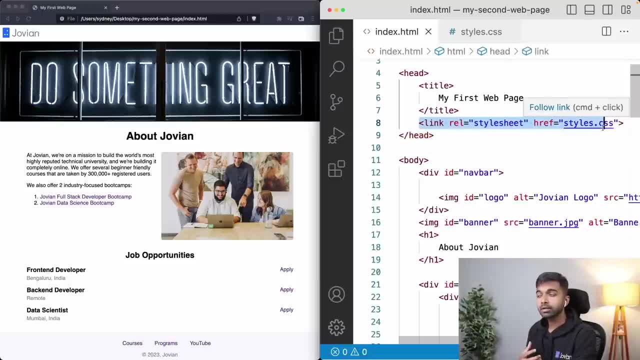 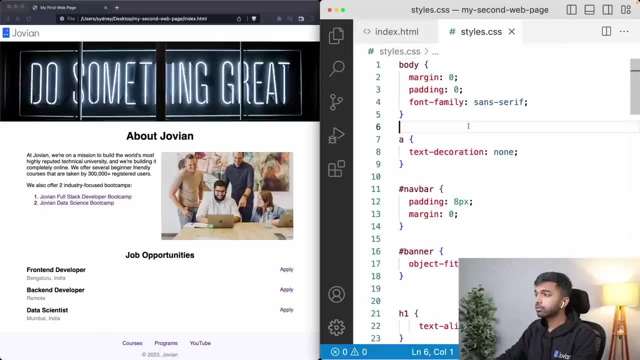 So there are many ways to attach CSS styles to HTML web pages and one which is called CSS styles. So there are many ways to attach CSS styles to HTML web pages, And one way to do it is by using the link tag and putting all the styles in a separate CSS file, which we have here. 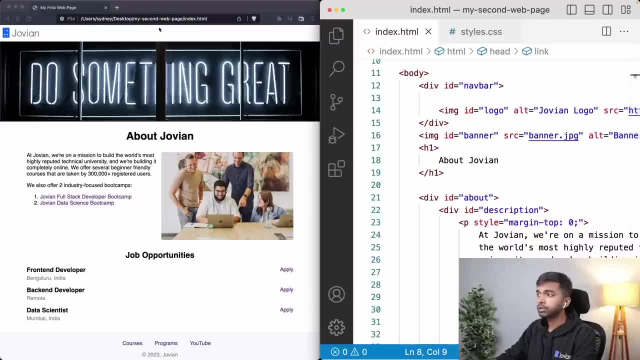 Then, of course, in the body itself, we have the nav bar over here, and this is all the code for the nav bar. So we have the nav bar, which is a div, and then an image inside it which is the logo over here. 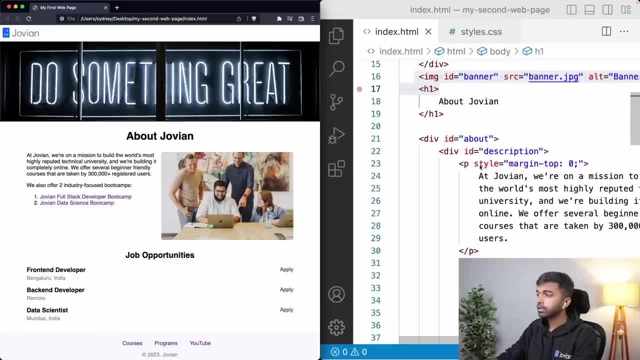 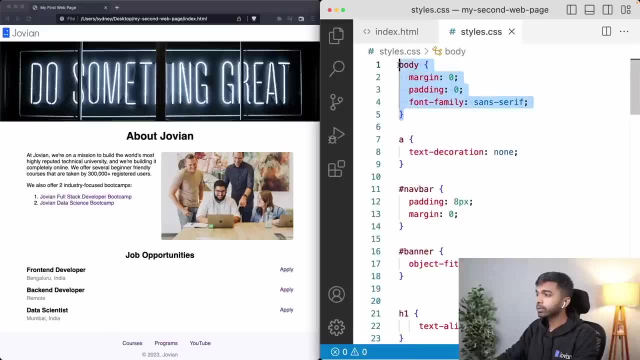 Then, of course, we have a banner, which is an image tag right here. Then we have an header. We have a header H1, which is right over here. You can see that all of these are styled as well. So we have the body. 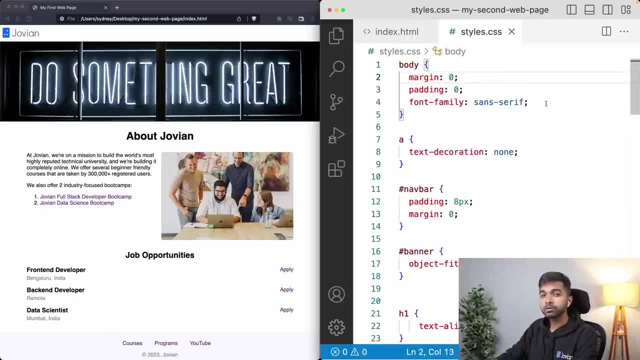 The body. we've set the margin and padding to zero and we've set the font family to sans serif. We've also set a text decoration for the nav bar. We've set up padding. We've also set a margin for the banner. 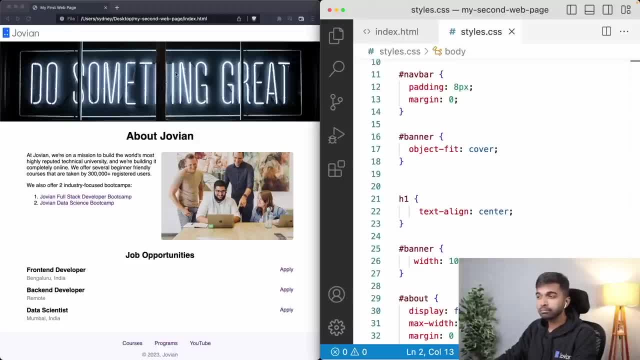 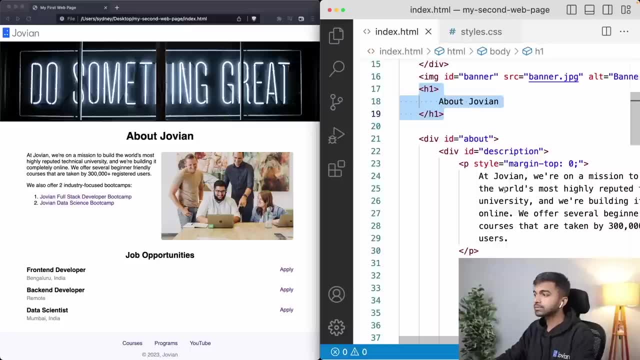 We've also set an object fit over here so that it goes up properly, no matter what the size of the pages. And for the header we've set the text line to center, So we've added various styles as well. Then we have this about section, and in this about section we have a left section and a right section. 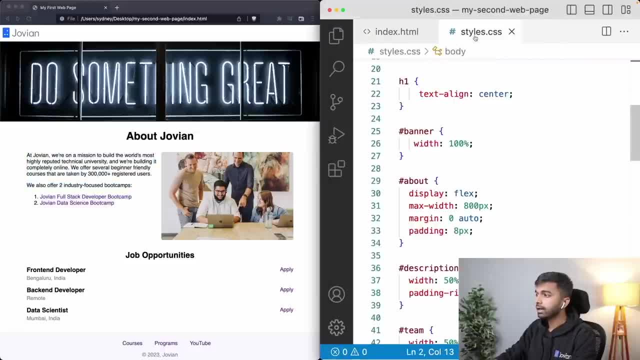 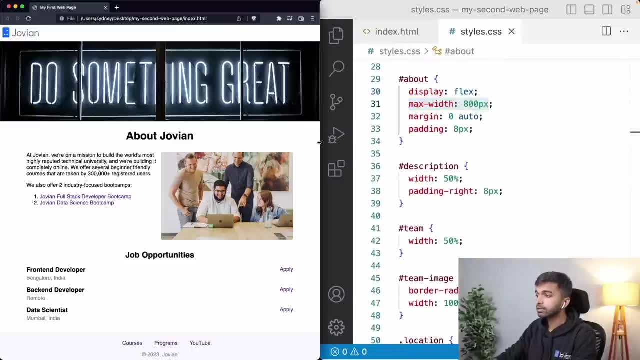 But the way we did this is: We have this about div and for this about div, we've set the display to flex And we have set a maximum width for this about div. So you can see here that the maximum width is ensuring that this about div doesn't become too big. 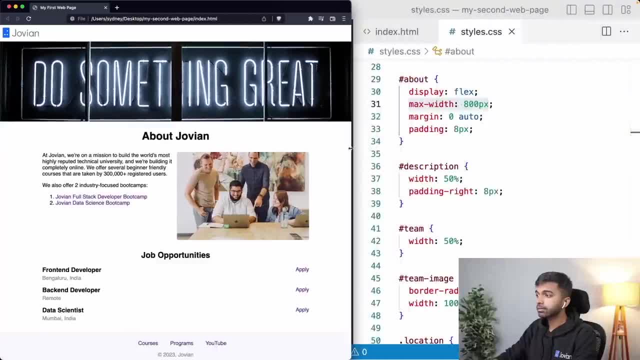 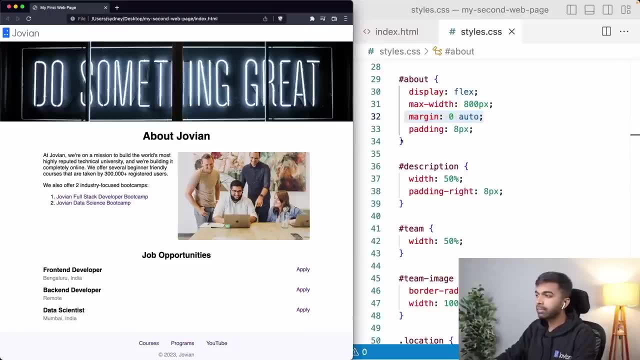 Apart from that, we've also set a margin that ensures that it is always at the center. Okay, So I'm going through this quickly, but review the previous lesson If not. if some of this doesn't make sense, we've also added a padding. 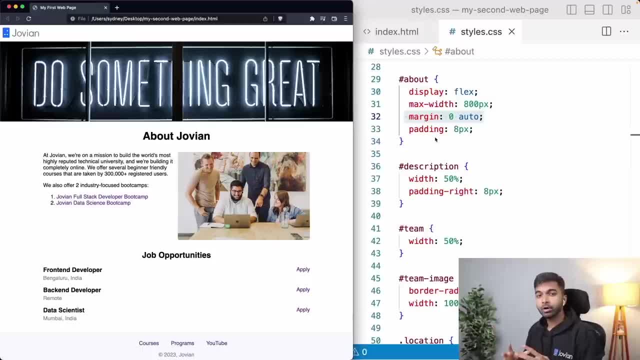 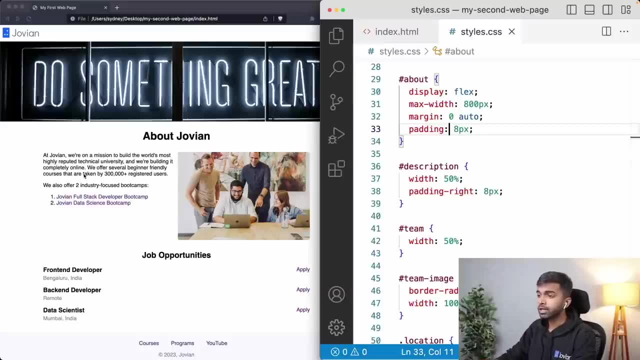 So remember the CSS box model: the padding is inside the border, The margin is outside- Okay, Outside the border. It's a good thing to practice and review from time to time. Then, of course, we have we have the description, which takes a 50% of the width. 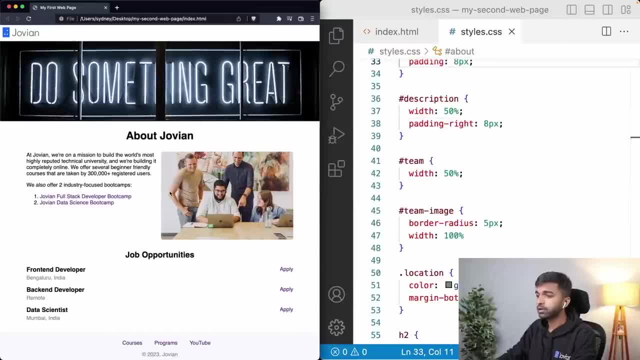 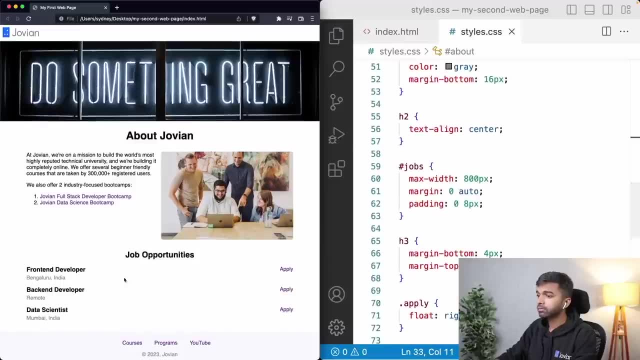 Then we have the team image, which again takes up 50% of the width, and the team image also has a border radius over here, And then we have these job opportunities. So we've used an edge to here. They can see we have the description. 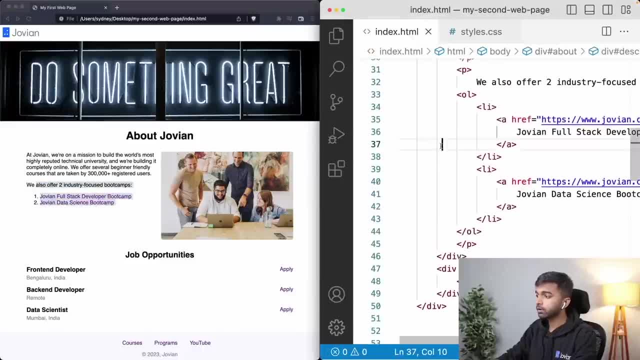 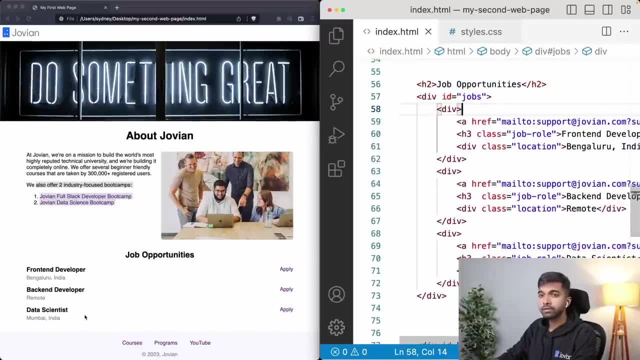 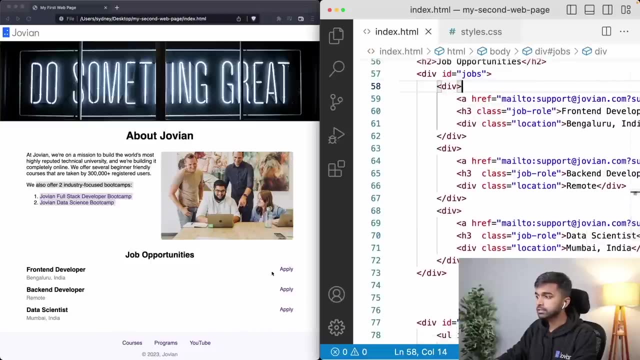 We have information about the two bootcamps which we have used- a list for a list tag- and then we have job opportunities We've used an edge to here. Then we have a div called jobs And in this div we have the three jobs: front-end developer, backend developer and data scientist. 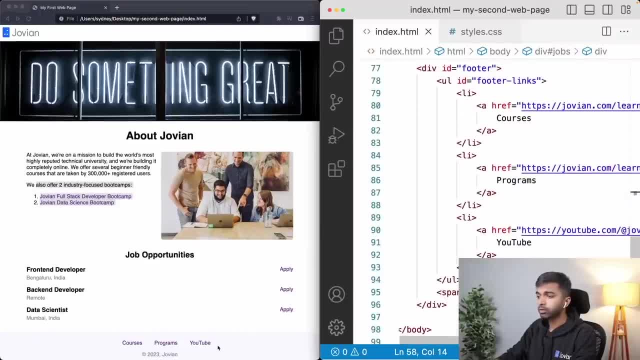 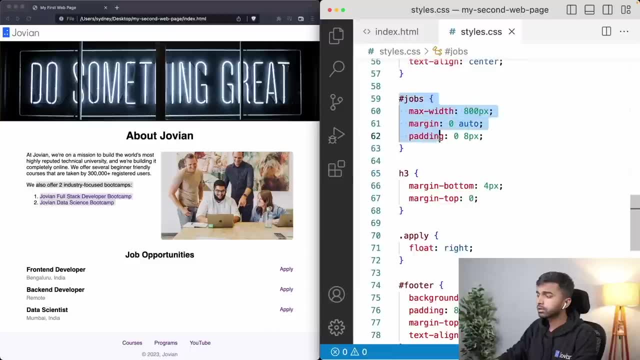 And finally, we have courses, programs and the YouTube link in the footer. Okay, Of course, there are some styles related to the jobs div as well. There are some styles related to each of the jobs we have. those are H3, and there are some styles related to the footer. 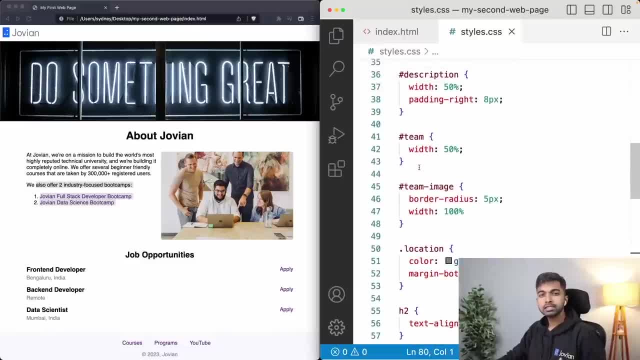 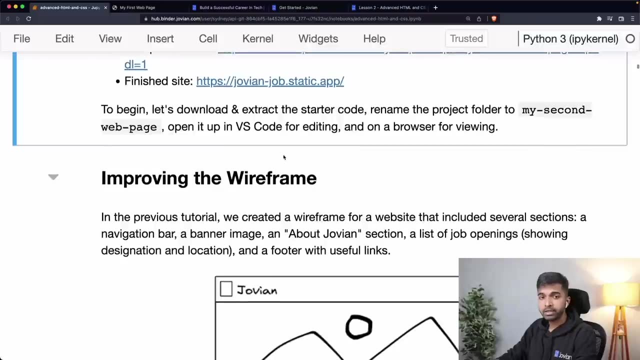 Okay, So very basic HTML and CSS that we applied and we, of course, deployed it to the cloud using a simple hosting platform where we could upload a zip file. All right, So that's what we have from the last time. So we've opened up the webpage, we've opened up the project in VS code and we have renamed it to my second webpage. 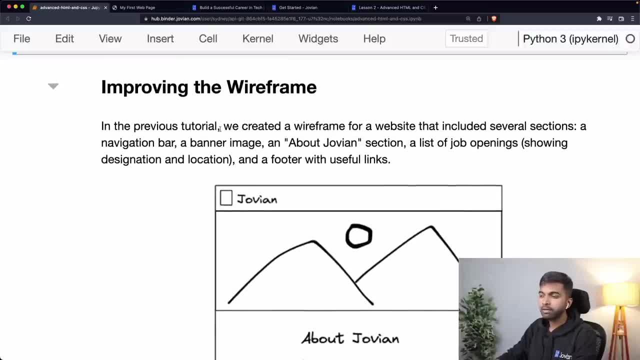 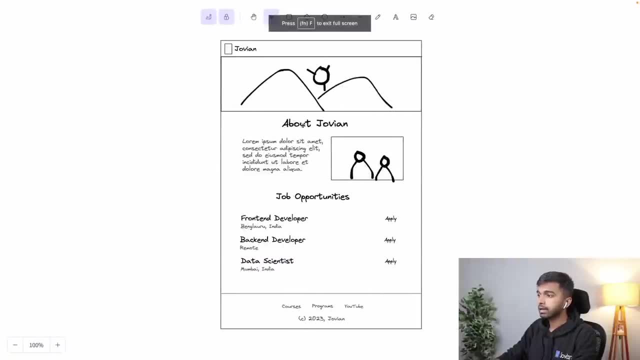 Now, the first thing we'll do is try to improve the wireframe. In the previous tutorial, we first created a wireframe. This is what it looked like, So Okay. So it contained this navbar banner and it contained the same sections that we have on the actual page. 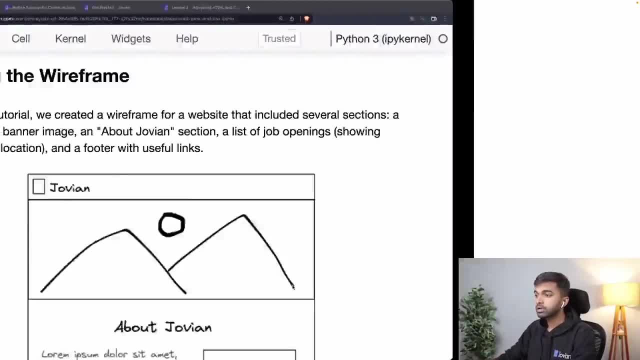 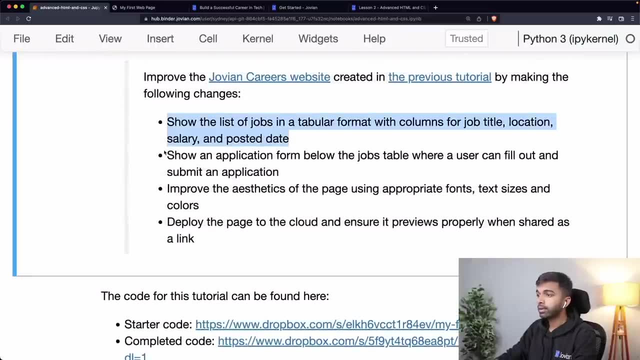 And we use this as a visual reference while creating the page. So now we are going to improve that wireframe, We're going to make sure that we are covering all of these things: a list of jobs in tabular format, the application form below the jobs, and also maybe the other things will follow, not necessarily in the wireframe, but when we implement them. 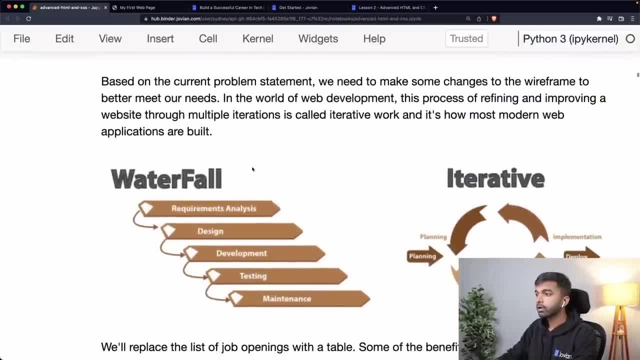 And this is something that you'll see as a very common practice in the world. So, in terms of web development, this process of improving the design of a web page and then going ahead and implementing it on an already live web page is called iterative development, and a website goes through multiple iterations, or even web applications. 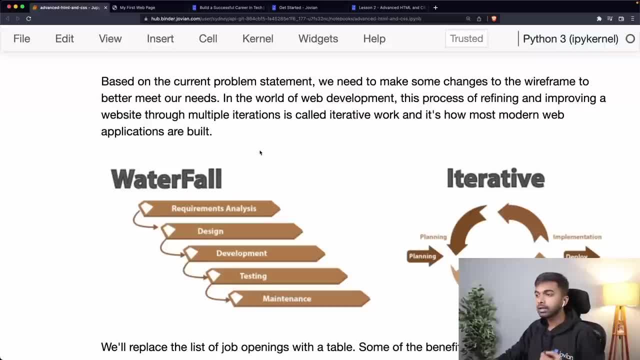 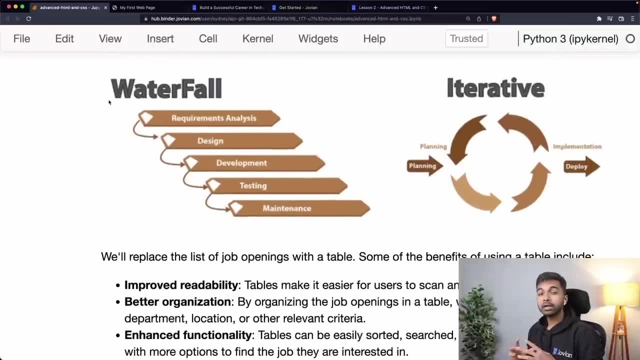 So when you look at Jovian, we add new features more or less every week, and that is how we approach building things. So the one approach that you could follow is something called the waterfall approach, where you identify all the requirements, Then you come up with a final design. 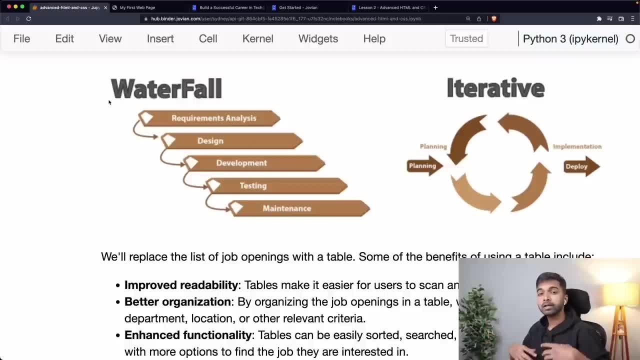 Then you do the development for the entire set of requirements at once, Then you test it and then you maintain it. That takes a lot of work and you often end up building a lot of features that nobody might use and missing out on some very important features. 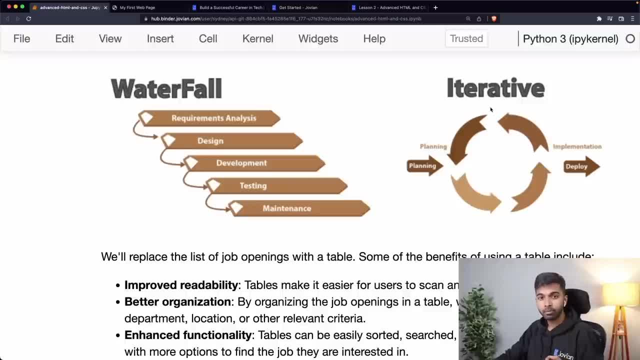 So another way to think about web development is to take an iterative approach. You should add the very least. push something out, deploy something that people can use every week or, if possible, every single day. So whenever you're building a website or a web application, you should think: okay, what can I build in a day that people can start using? 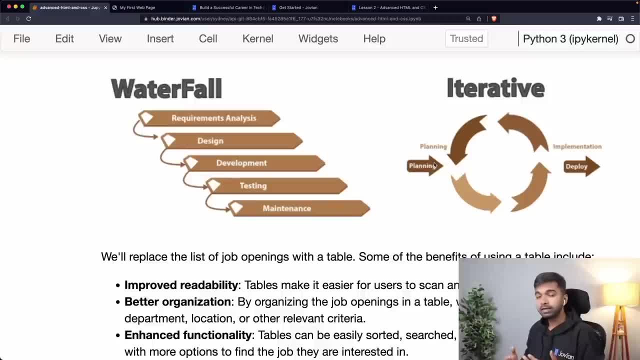 Well, however, you can do this. If you add a new feature to it, you can see that the job has been completed. It is, which is what we did the last time, And then, once people start using it, depending on their feedback, depending on what else you have in mind and how much time you have- try to come up with a second version with a new set of features and repeat that process. 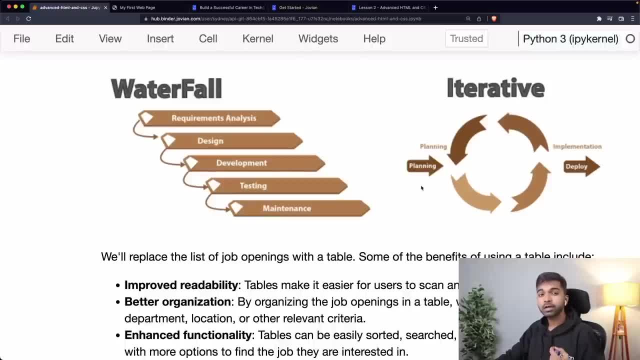 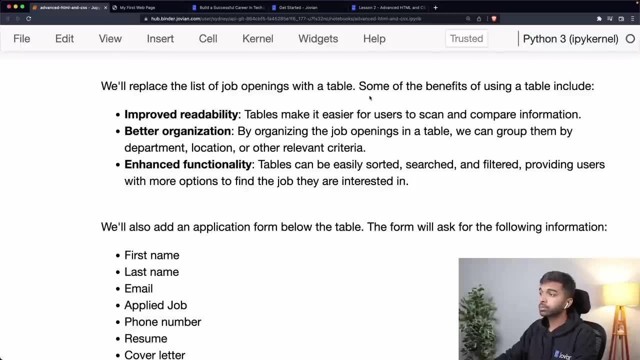 So iterative development is a very common practice in modern web applications, So this is something that you should get used to. So there are a couple of changes that we are making today. The first thing is to- And some benefits of the table are they: it leads to an improved readability, because tables 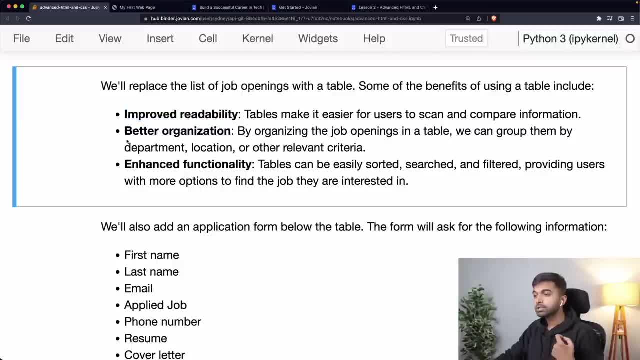 make it easier for people to scan things visually. Tables also offer better organization. So because organizing them in a table, you can also group them by department, location or other relevant criteria. later on, when we implement more interesting tables, And then tables can also have things like sorting, searching, filtering, et cetera. 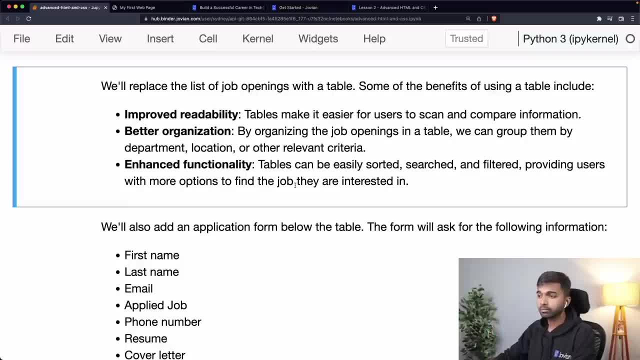 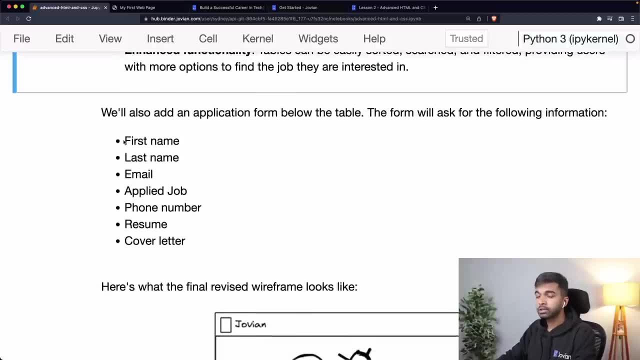 which we look at once. we look at web application development later in the program. Apart from the table, we'll also add an application form below the table. So the form will ask for the user's first name, last name or maybe the name as a whole. 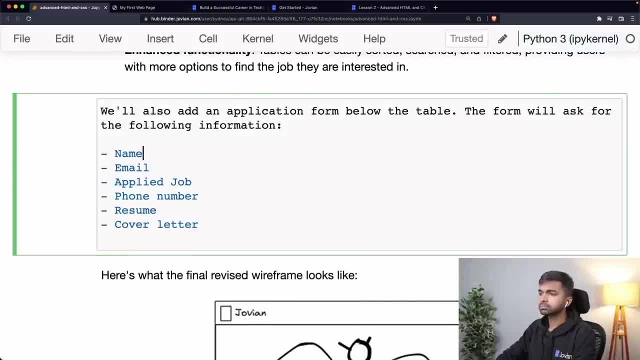 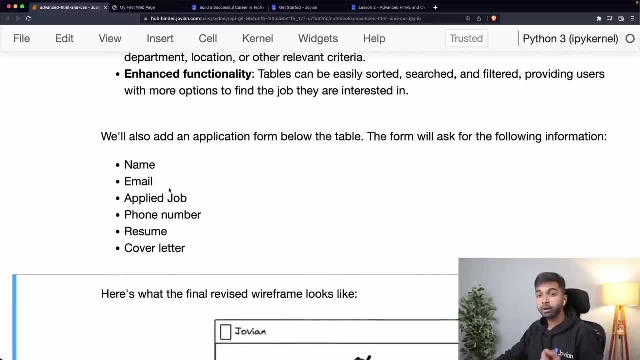 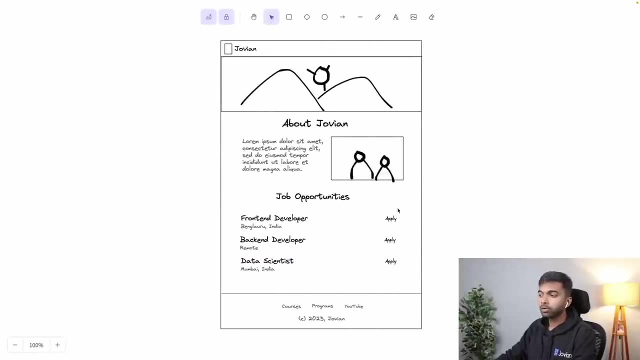 Let's just change that to name. So the form will ask for whoever is applying. The form will ask for the applicant's name, email, the job that they're applying for, their phone number, their resume and a cover letter. And here's what you can do. 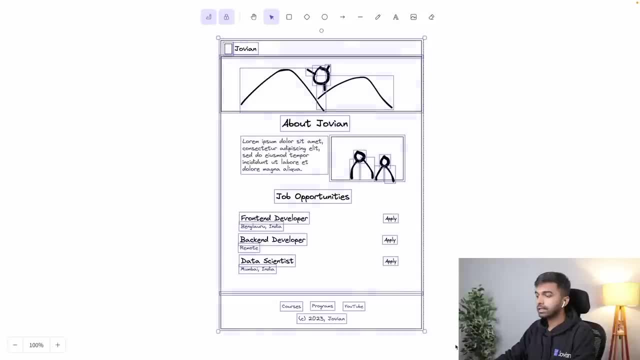 You can actually start revising the wireframe here itself, So you can take this and then create a copy of it and then paste it and then start moving things around. For example, you could get rid of, you could get rid of these, and then you could insert. 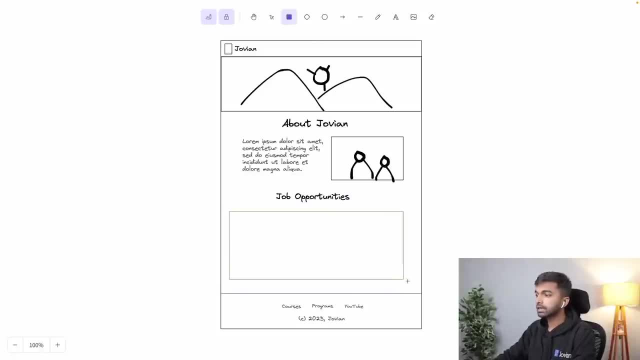 a table here, So I could, for example, go like this and create a table, and then I could make some more changes. Let me change that to black. Yeah, So I, for I could, for example- Yeah, For example- create a table here and then into that table I could add various columns. 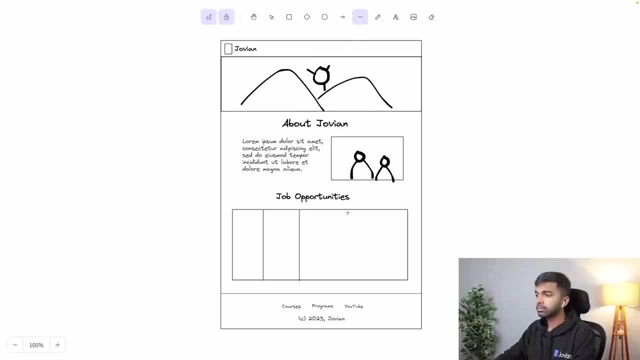 like this: So here's one column, is a second column, Here's a third column, And then I could start adding rows within the table And then I could maybe start adding information like job title. So these would be the column headers, And after adding the column headers, I can also add some data within those columns. 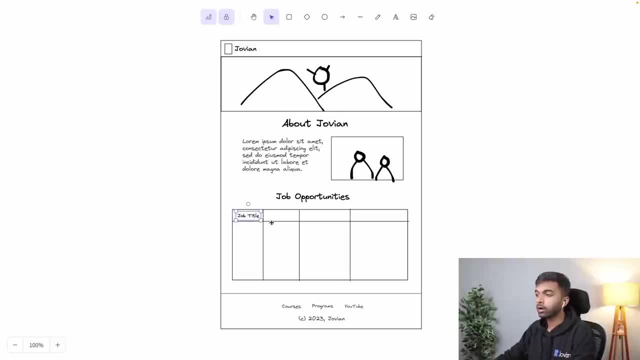 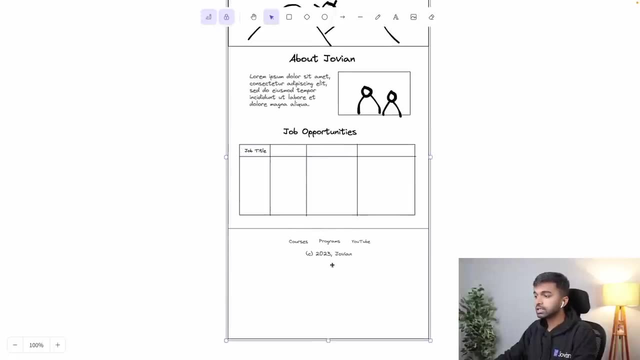 So this is how you enhance your wireframe. You are visually trying to put together what you want. What do you want your next version of the wireframe to look like? And then you could also go ahead and maybe extend this a little bit. 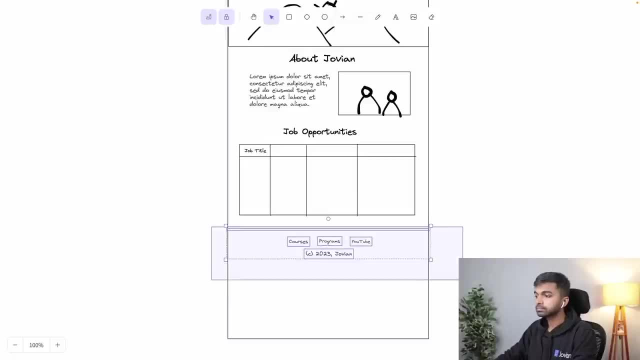 So move all this forward, Let's see, let's move all this down and you could then add an application section. So you could add a section called submit your application And then you could go ahead and maybe add a various input fields. For example, you could go ahead and maybe add a various input fields. 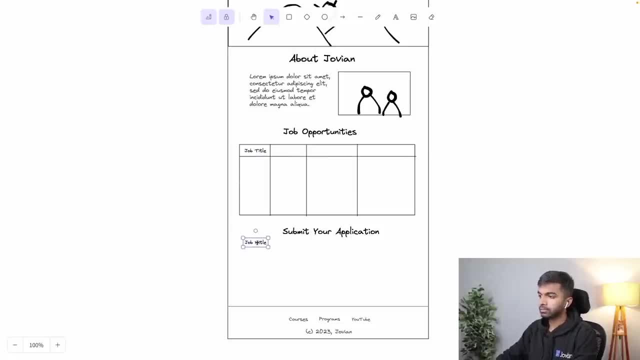 Okay, You could get an input field called name here And put an input box below it And then just create multiple copies of that to create the other input fields and so on, And you could add, maybe, a submit button somewhere at the end. 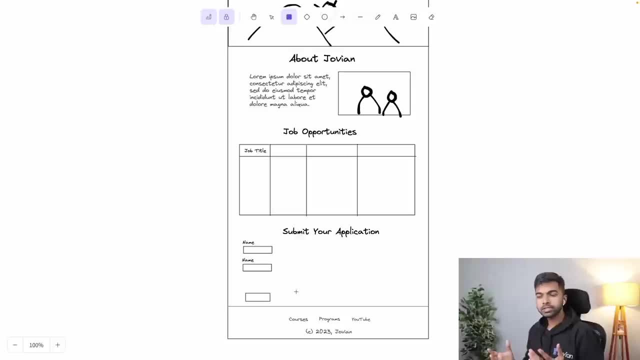 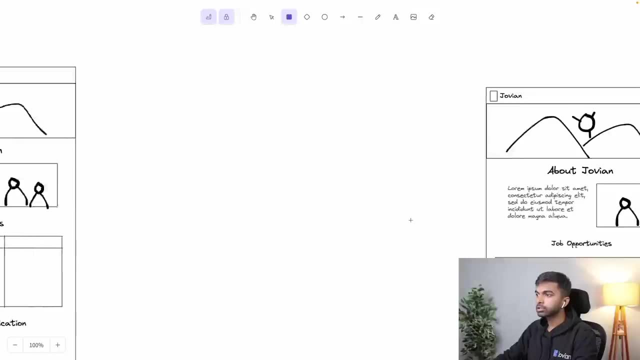 Right. So this is how you enhance a wireframe: just create a copy of your existing wireframe and keep adding new things, new sections, before you go out and start coding. Now I've already done this, So I'm not going to show you how to do that. 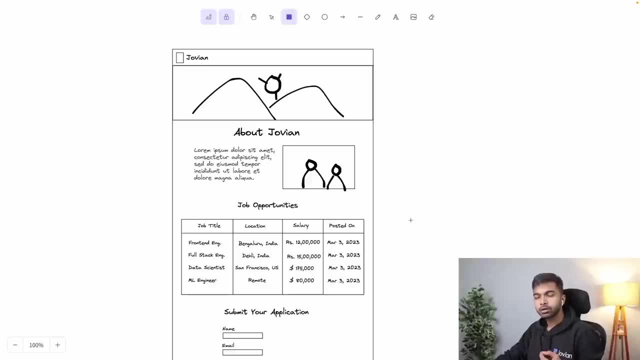 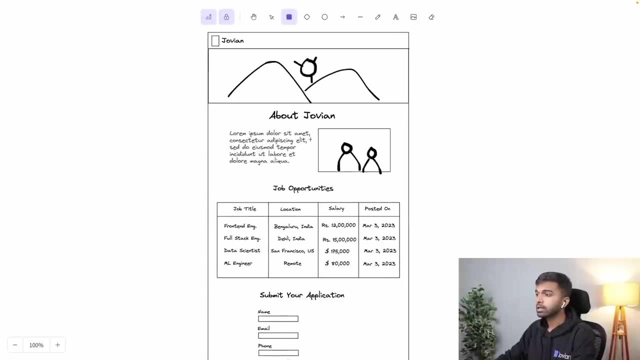 I'm going to show this entire process to you, But I encourage you to just do it all yourself. Get into the habit of creating quick wireframes before you start writing HTML code. that will save you a lot of time while coding. So here we have added a job opportunities table. 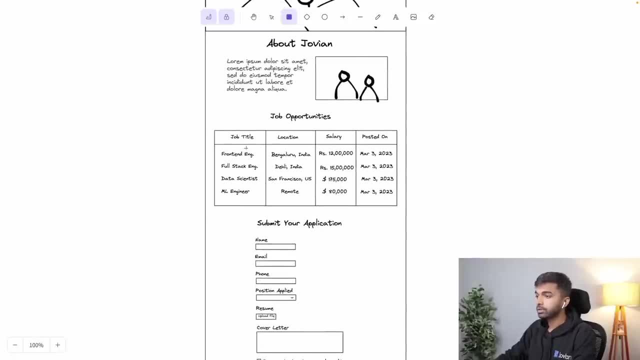 And you can see that we have a job title, location, salary and posted on We have the job titles, we have a bunch of locations, we have salaries both in Indian rupees and in dollars, And then we have a poster on date. 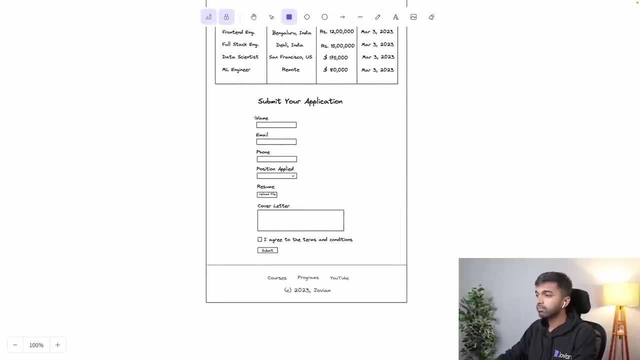 And below that we have a submit your application form And in this form we ask for a job title, We ask for the name, email phone number and there's a drop down here asking for the position the user has applied to. 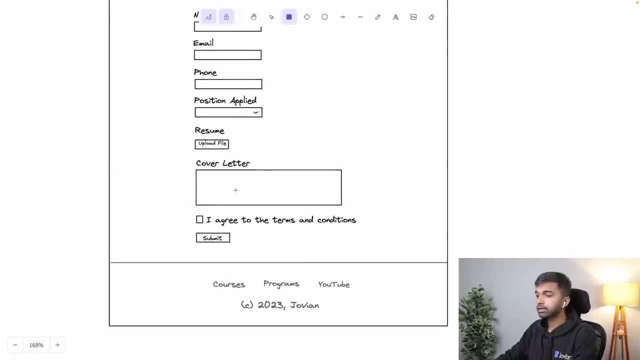 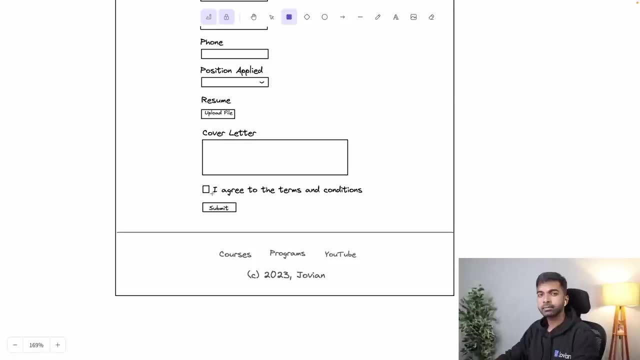 And then there is a cover letter. there's a box here for submitting a cover letter, Okay, And there's also this checkbox here that we're asking the user to agree to the terms and conditions, which is to be contacted by us or for their resume to be shared within our 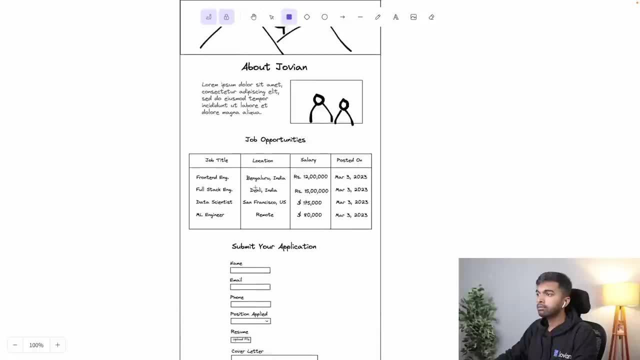 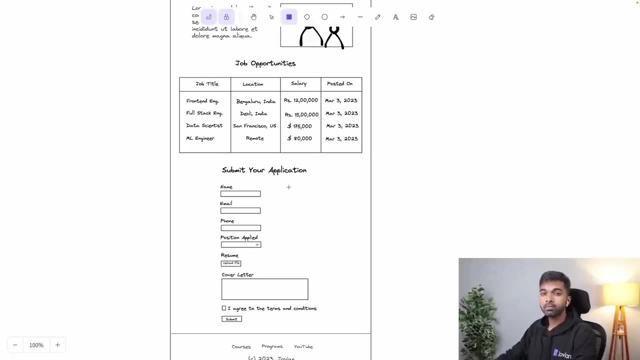 company and so on, And there's a submit button. So now we have a clear idea of what we want to build today. specifically, these are the two sections that we want to work on today. First, of course, we want to make them aesthetically pleasing. 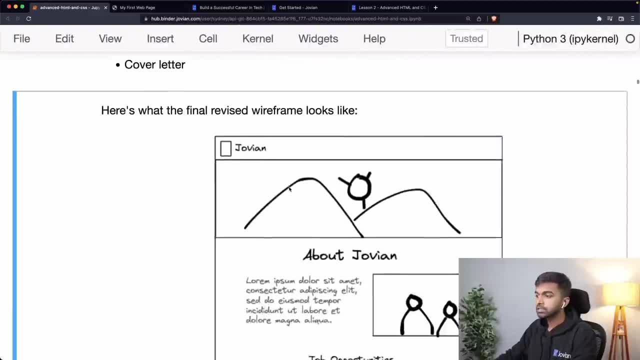 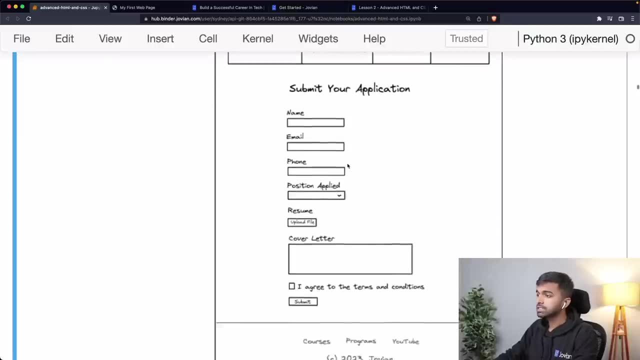 And then we also want to make some other changes to the site in general. So this is a revised wireframe. we still have the navbar banner about section, but now we have a job opportunities table And we have a submit your application form. 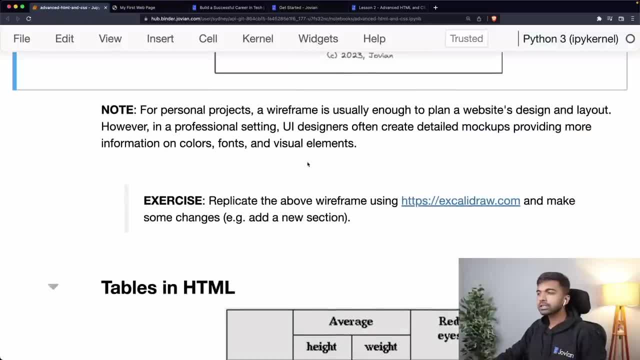 And of course, we have the footer as well. Again, for personal projects, a wire frame is usually enough to plan a website's design and layout, But in a professional settings, UI developers will often create detailed mockups providing more information on colors, fonts and visual elements. 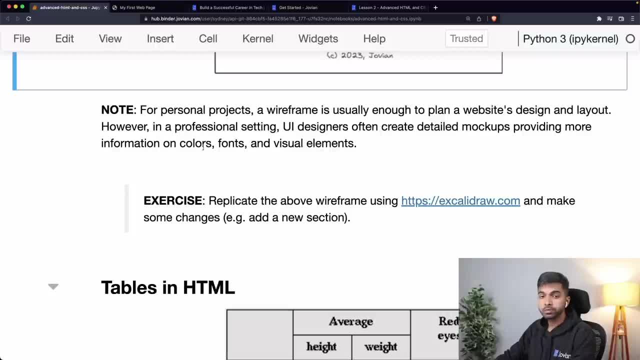 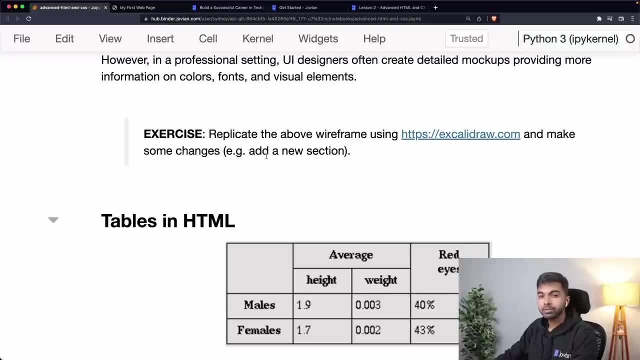 And this is an area that we're going to be covering in a few minutes- that you can work, that you can use while actually coding the web page. So, as an exercise, I encourage you to replicate this wireframe and maybe also add some new sections. see if you can add a new. 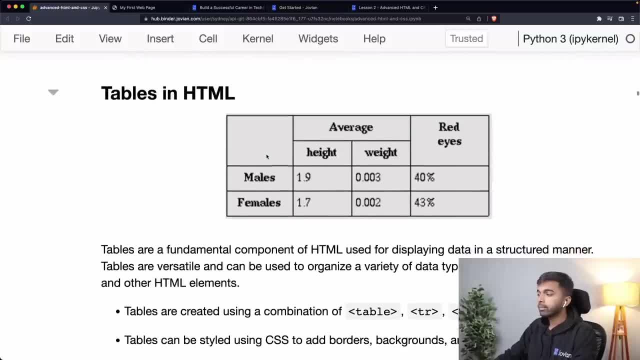 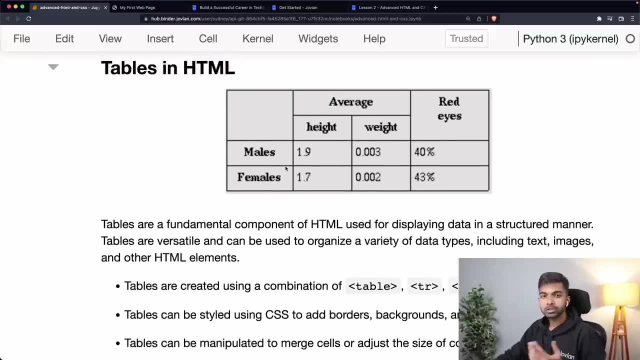 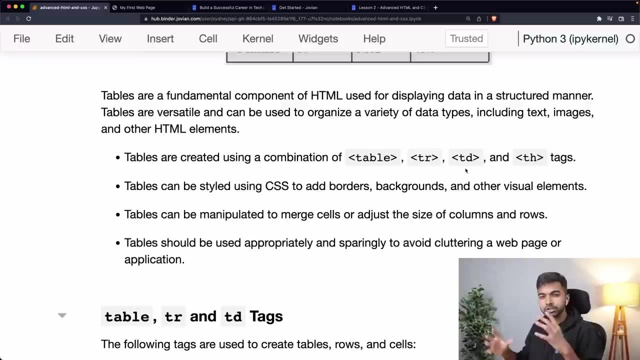 section and implement that while you're working through this lesson. But let's come to tables in HTML Now. tables are a fundamental component of HTML used to display data in a structured manner, And tables are created using a combination of the table, tr, td and th tags, So there are a bunch of 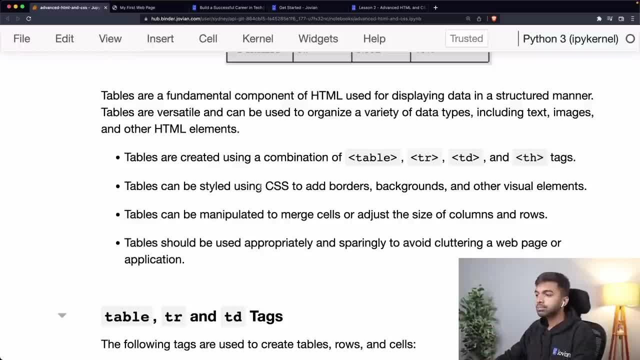 tags that have to come together for you to create a table, And tables can be styled using CSS, just like all other HTML tags, to add borders, backgrounds and other visual elements. It was can also be manipulated to merge cells. So, if you see, here it's not just a simple table with rows and 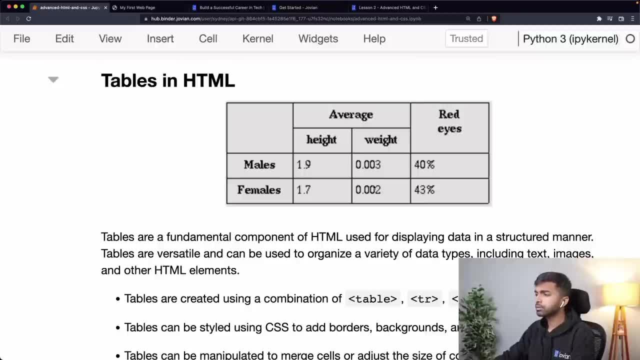 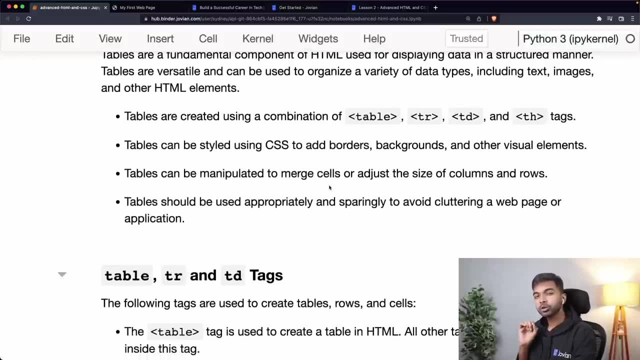 columns, you can see that these two are merged, And then these two are. this is vertically merged as well. They can do lots of interesting layouts with it using tables, But I do want to mention that table should be used appropriately. don't put everything within a table you might get. 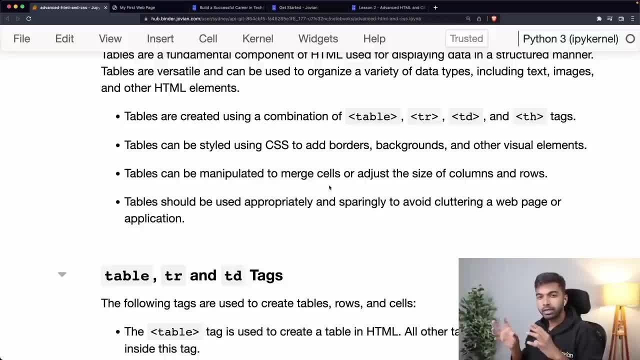 this temptation to just use a table for the entire web page to lay things out, But that's not a great idea. you should be using CSS for layout, and tables should be used only when you want to show a grid of data which fits in neatly into a table. So a good rule of thumb is if something can be represented. 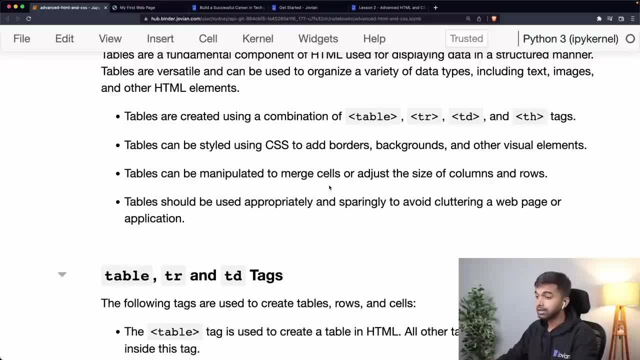 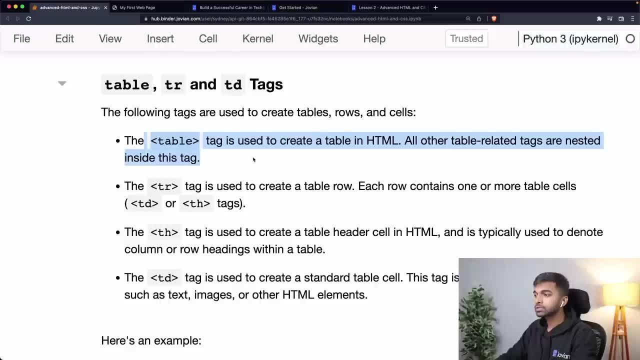 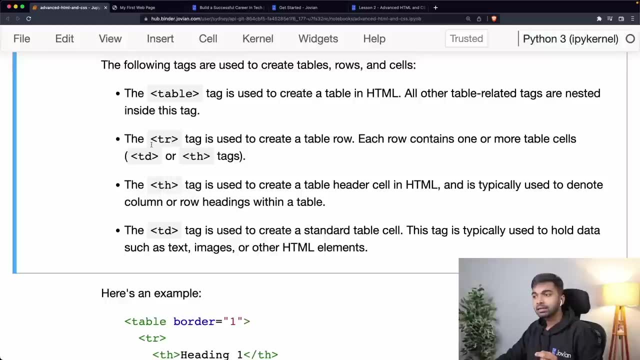 using a spreadsheet, then a table is a good way to represent it in HTML. So a table is created using the table, tr and td tags. The table tag is used to create a table in HTML and all other table related tags are nested inside this tag. then the tr tag is used to create a table row And each row. 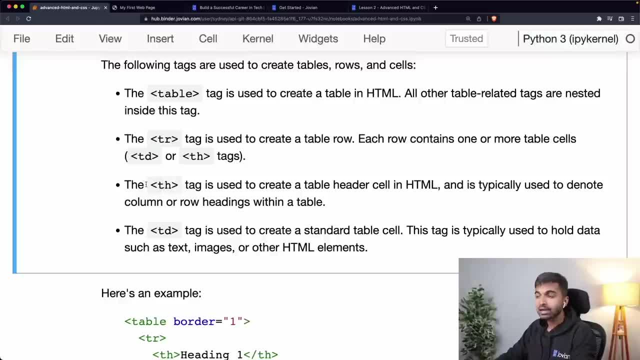 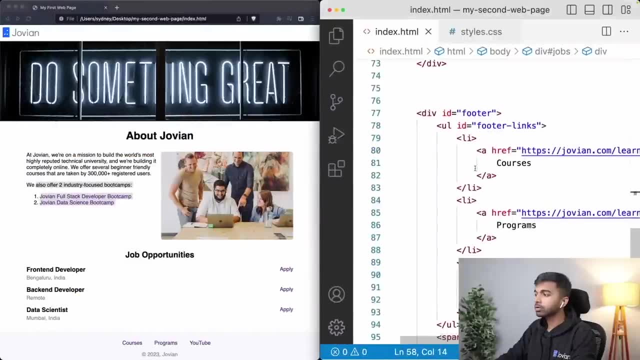 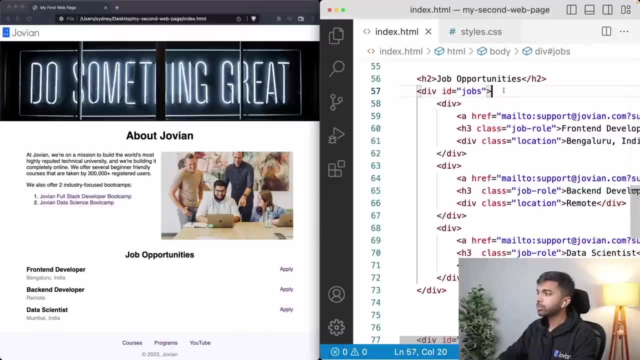 contains one or more table cells, And the table cells are created using the th tag and the td tag. Okay, so let's see these in action And it will start to make a lot more sense. So the first thing I'm going to do here is go down and find the section job opportunities, And I'm going to remove 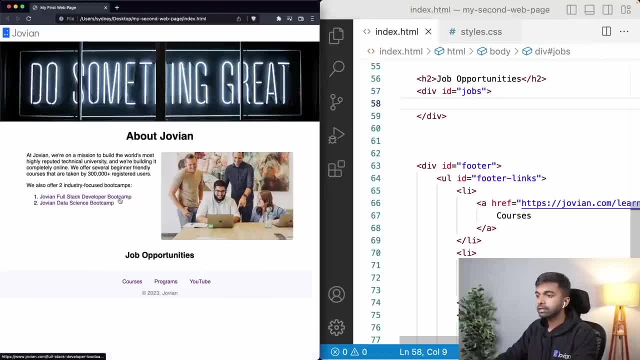 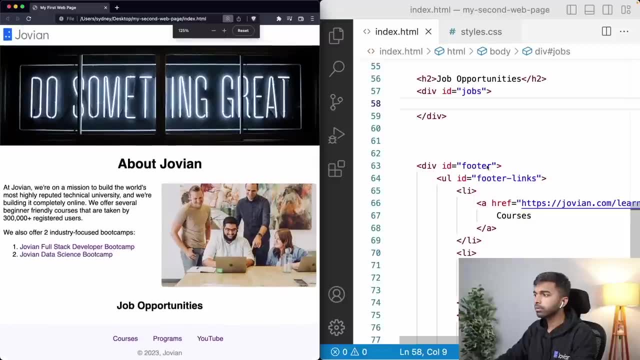 this div containing job opportunities And I'm going to remove this div containing job opportunities, And if I just reload here, you can see that now we no longer have job opportunities on this page. Let me just zoom in a little further. Okay, now let's start adding a table here. So let me add a. 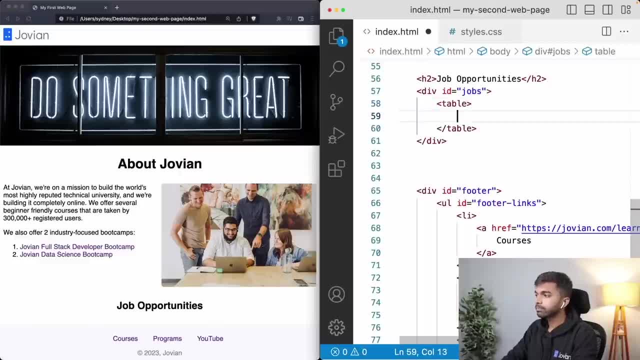 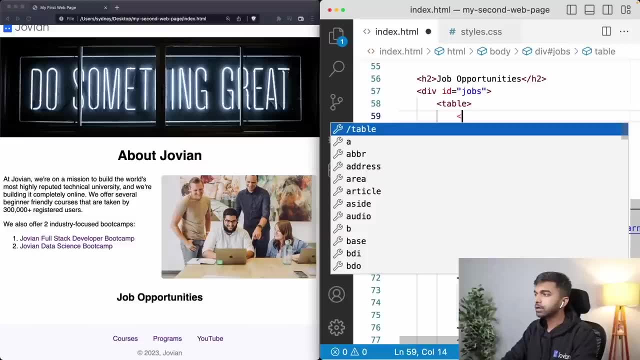 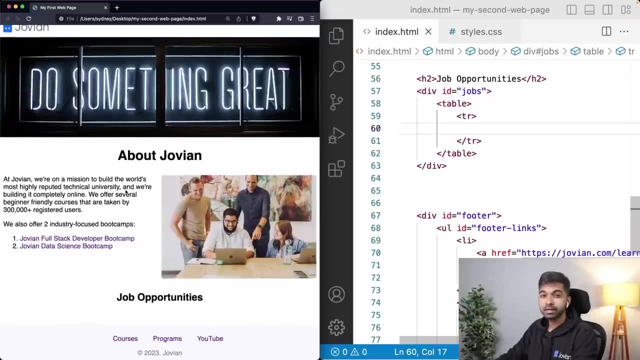 table. Okay, and let me save that, And you can see nothing really happened. some additional space got added, But the first thing I'll do is I'll add a row within the table. So a row is added using the tr tag And let me save that, And still nothing happens. 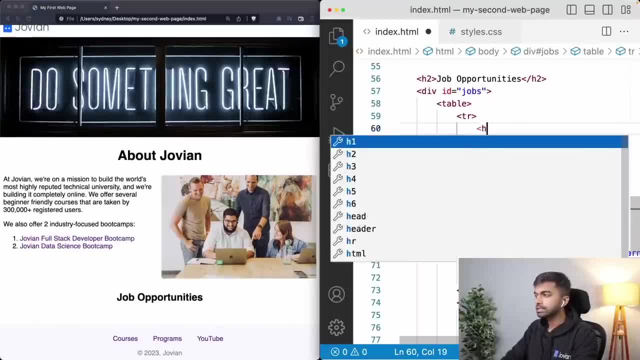 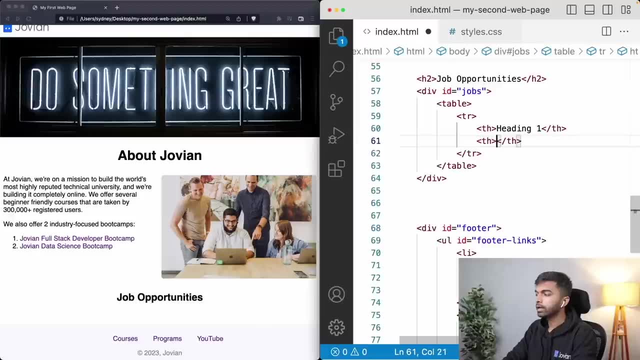 Now let me actually put some heading. So let me create a heading called heading one. So I'm going to create two column headings, one called heading one and one called heading two, And these are created using the th tag. Okay, So now you can see over here in the corner, we have heading one. 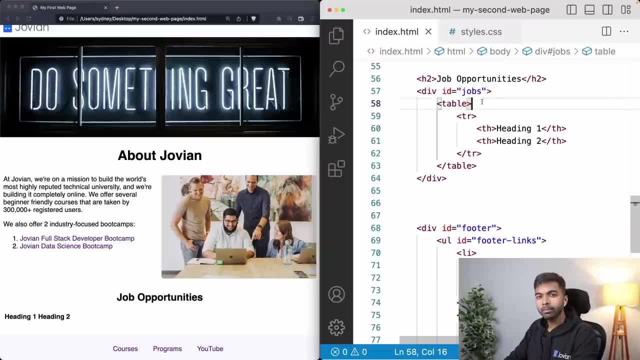 and heading two, And normally you might want a table with a border. So one quick way to add a border for a table is just by specifying the border attribute. Okay, Now, once I've added a border, you can see that there is a border around the entire table And 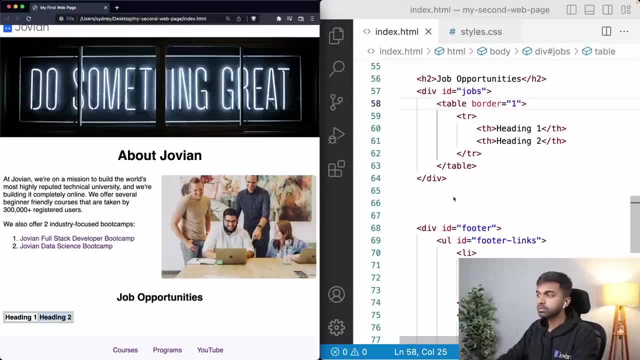 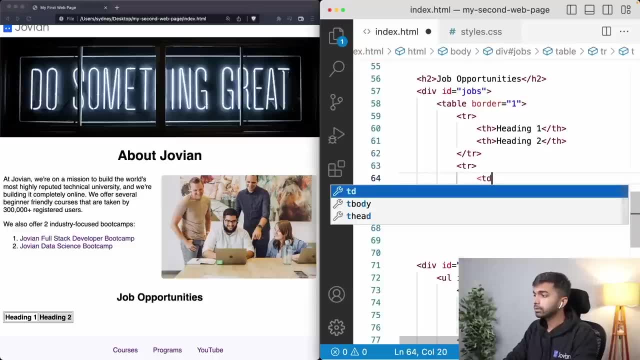 then there is a border around heading one and there is a border around heading two as well. Okay, let's add more rows within the table. So let's add a tr. Now let me add another element. So now I'm no longer adding headings, now matching, and now I'm adding actual data elements. 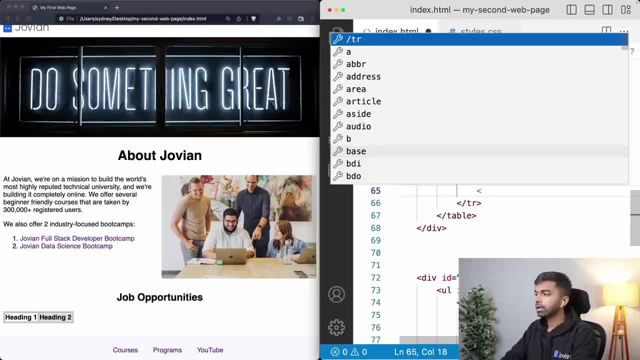 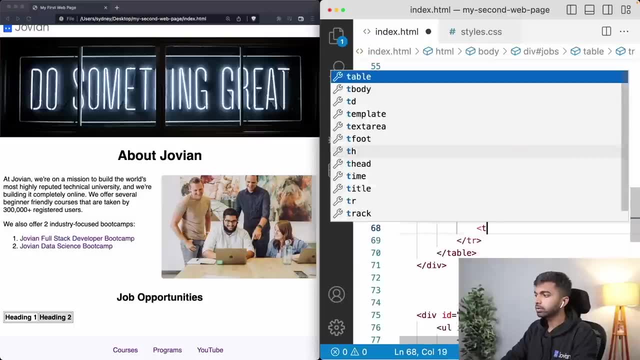 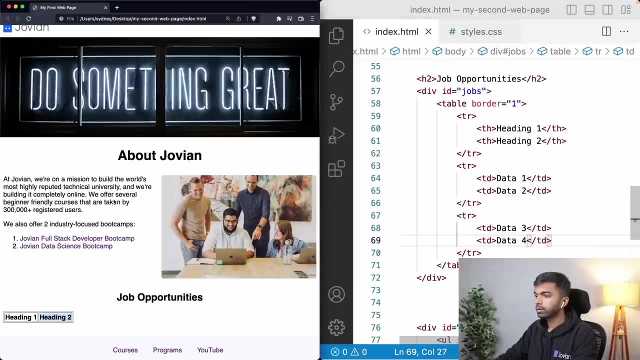 Okay, so I'm just going to call it data one for now And TD data two, And let me just replicate that for one more row: AD data three And TD data four. Alright, so now we've created a table successfully. I hope you can see it, you. 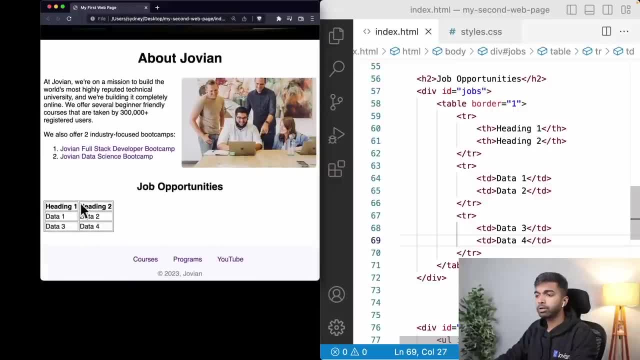 it's right here in the bottom left corner of the web page. And now, now that you've understood how tables work, we have this table tag And in this table tag we have a row. this is the header row, and that contains these th tags. so th is header. then we have these more rows and in these rows, 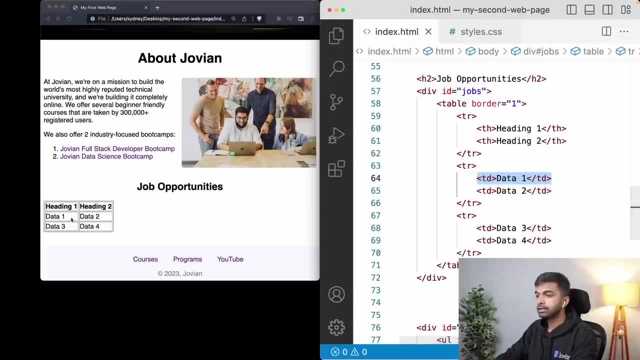 we have the td, and td creates normal data. so you can see the difference between the heading and the normal data is that the heading is bold, and if the table was bigger you would also notice that the headings are centered, but the normal data is left aligned. so that is a difference, but it's also 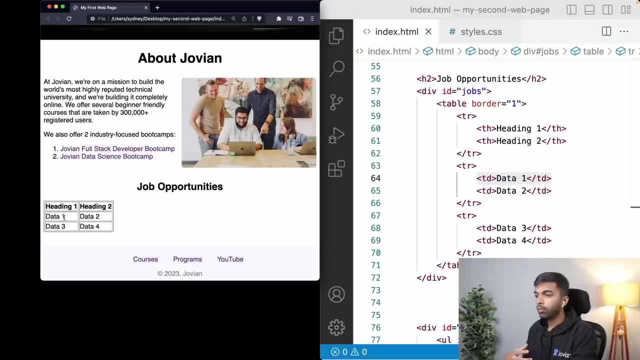 semantically informing the browser what is the heading and what is just data within the table. it is also used by screen readers and search engines to identify the structure of the table. okay, now i encourage you to experiment with the table. what happens if, for example, i put an? 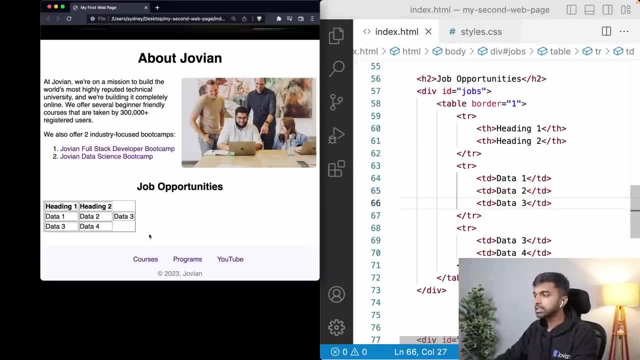 additional column here. let me just save that and you can see that a new column got added here. but they you don't have that same column here available and that is why you have empty space here. or what happens if let's say you have like a stray td somewhere. so let's say you have this. 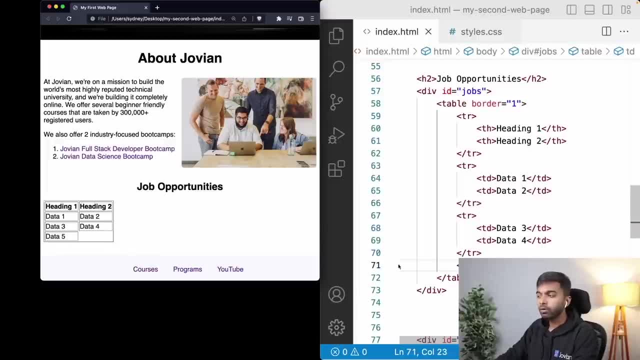 data 5 somewhere. what? what does that do? so that's why you have empty space here. or what happens if, let's say, you have, like a stray td, so that creates a new row, even though you do not have a proper tr. so even if you do not have a 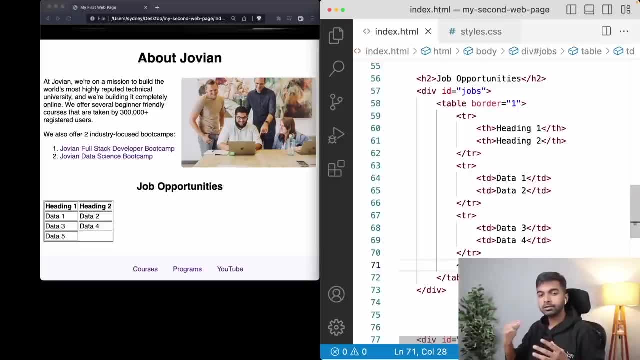 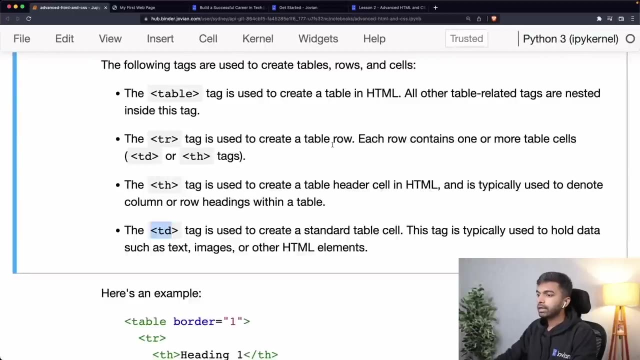 perfect structure of table and then tr and then th or td. most browsers will still render your tables, but it's a good idea to maintain the proper structure while building a table. okay, so that's how you build a table in html, fairly straightforward. okay, so let's maybe go ahead at this point. 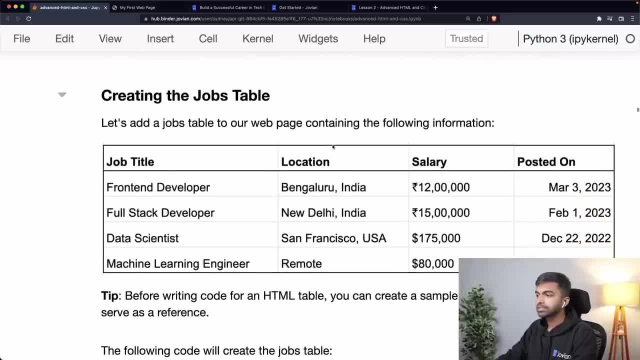 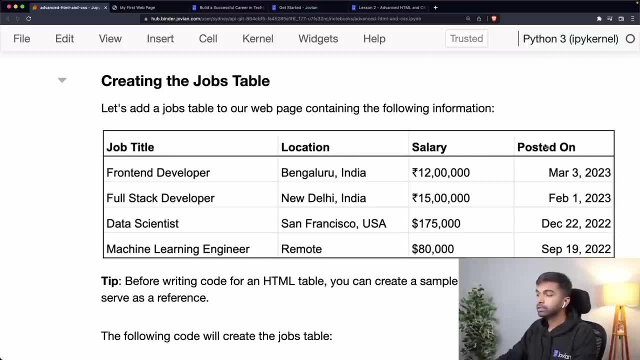 and let us add this data into a table. so we want to get the job title, we want to get the location, we want to get the salary and we want to get when the job was posted. now here's a quick tip for you. whenever you're building html tables, it's always a good 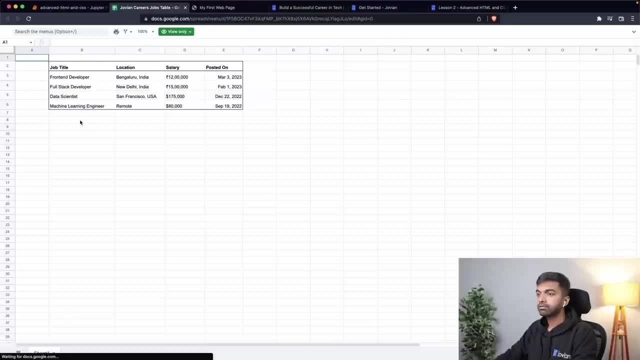 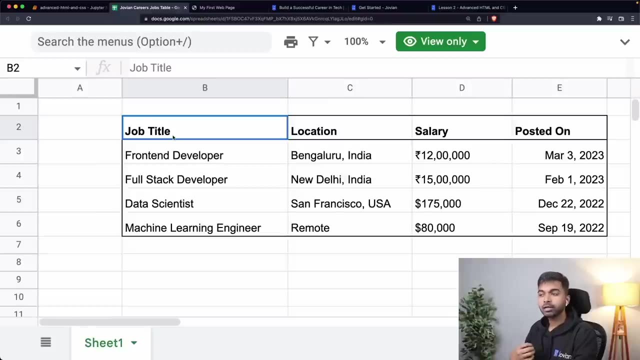 idea to first maybe create a spreadsheet, like i've done here. i've created the spreadsheet- let me zoom that in a bit- and i am simply going to now use this spreadsheet as a reference for creating the table, and i can also just copy paste the data very easily from the spreadsheet onto the table. 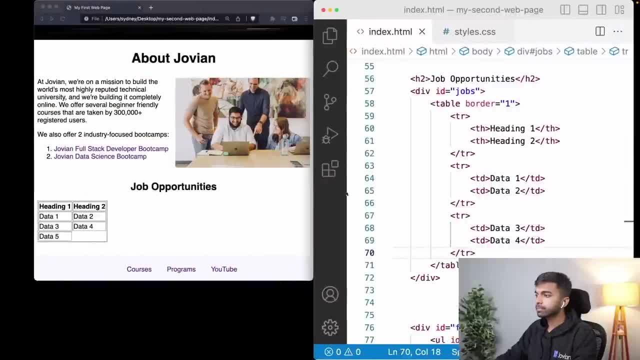 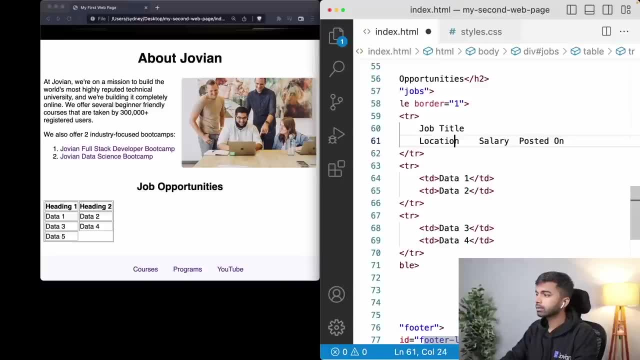 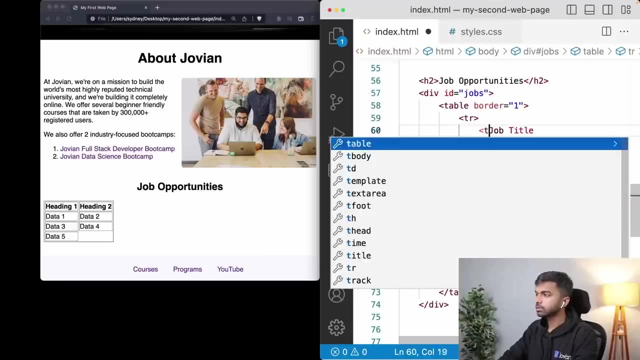 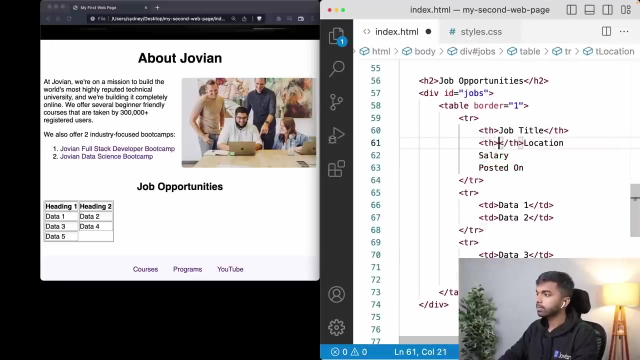 so let me just go in here and copy the table headers and now i am going to paste in these headers. so my first row is going to be a row of headers and that is going to contain these th tags. so now we have a th for job title, we have a th for location and we have a th or table header for salary. 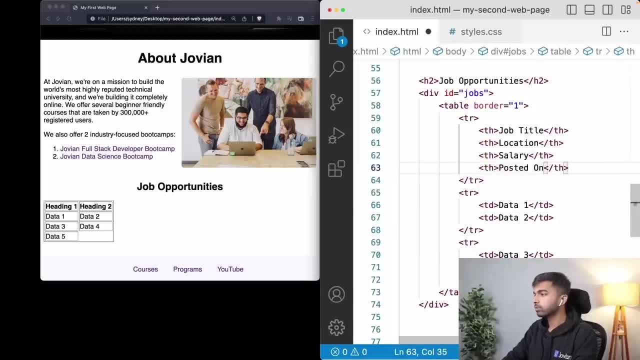 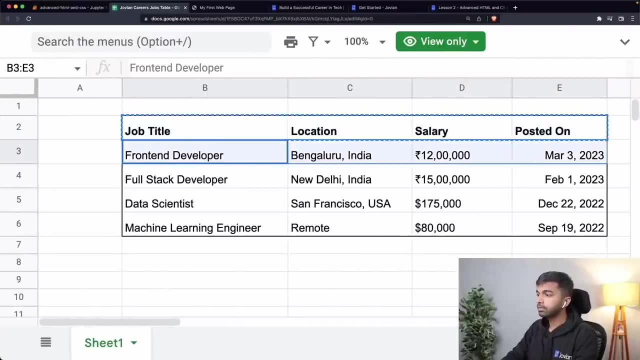 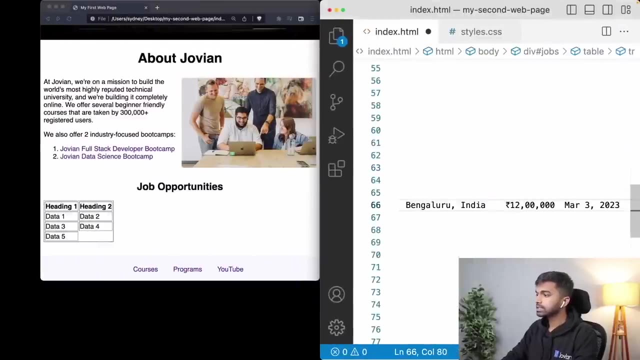 and finally, we have a th or table header for when the job was posted. great, now let's start adding the jobs one by one. so once again, i'm going to go in and copy this front-end developer bengaluru. i'm going to copy the salary and the posted on date as well, and let me get rid of these and paste that in here. 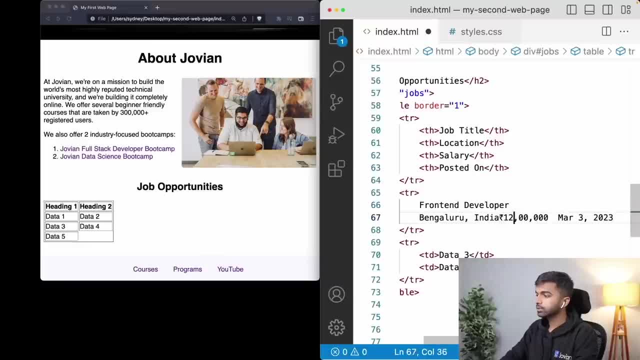 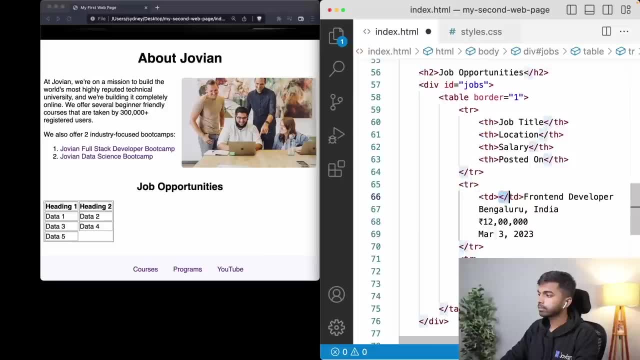 let's bring that into new lines over here, okay, and let's put in a td here. so again, wrap the data inside a td and you don't just have to put simple text. you can put entire lists, you can put paragraphs, you can put whatever you want, you can put images into a table, but for 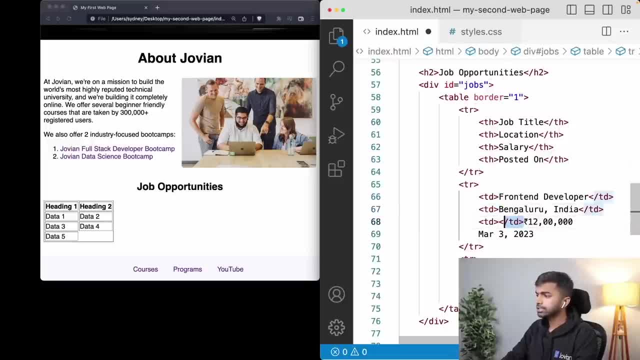 now we'll keep things simple. we are just going to put some normal text into each table cell. so each box that you see within the table is called a table cell. so that is something that you will notice in the terminology, especially if you're searching for questions online. okay, so that. 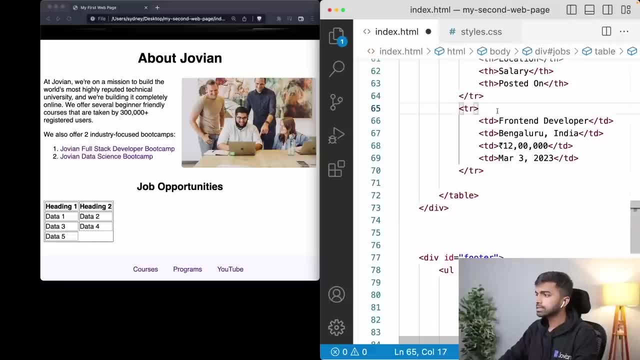 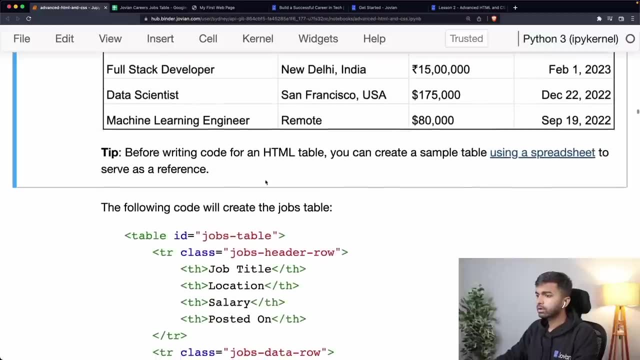 is the second job role. let me just grab the table and i'm going to put in the table cell. so that is, grab this and create a few copies of this and in fact what i'm going to do is also give it a couple of classes. so i'm going to give it the class, i'm going to give the entire table an id. 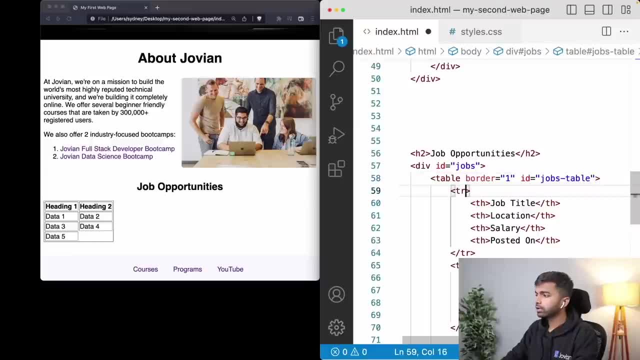 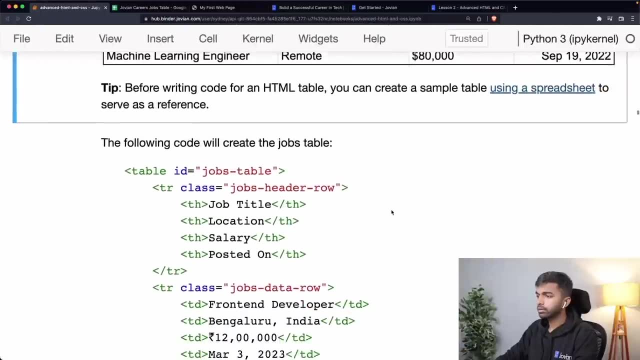 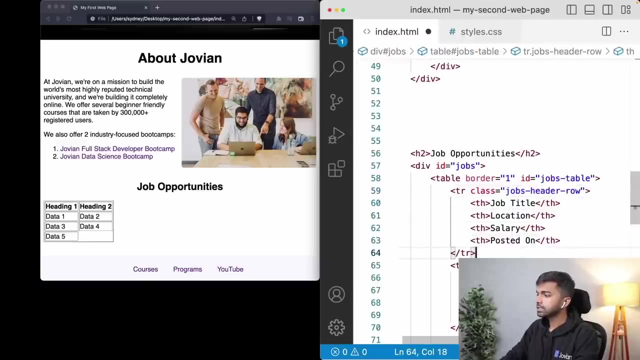 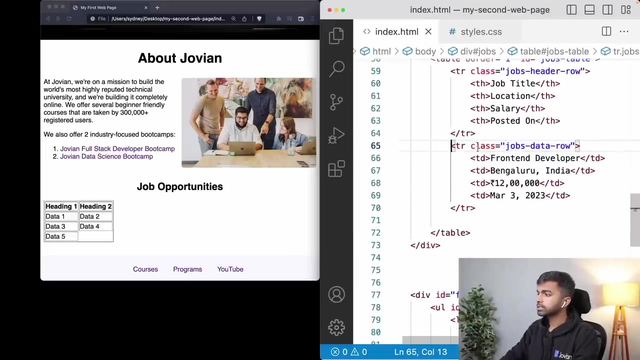 jobs table and i'm going to give this a class jobs table header and or jobs header row. let's just call it jobs header row and let's give this a class jobs data row, okay, and let's create copies of this. so we are adding the classes because we're going 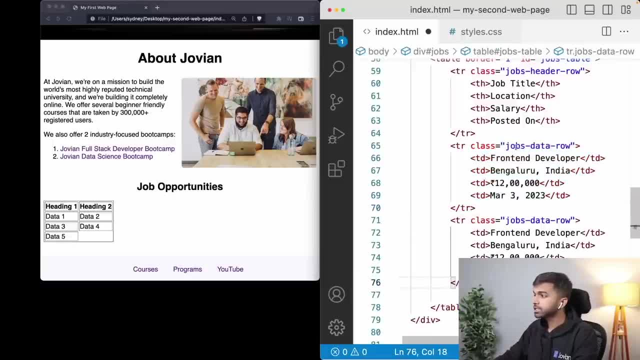 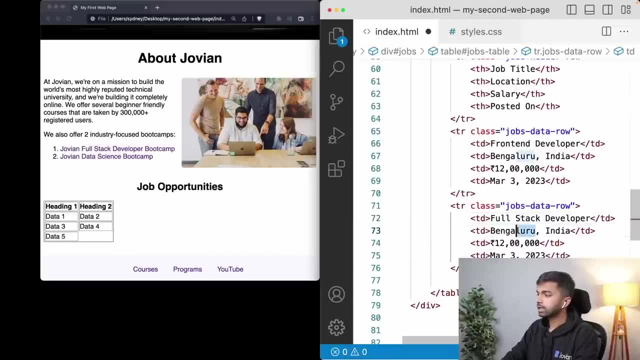 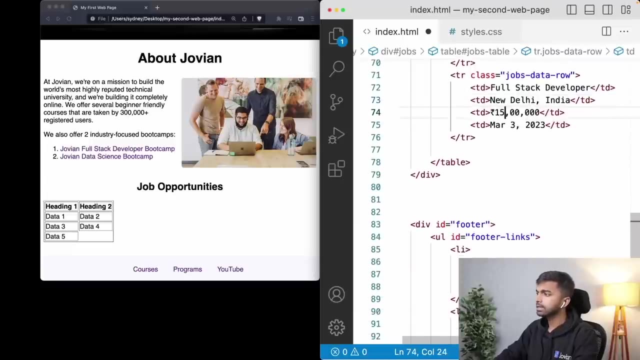 to use them later for styling. now we have the jobs header row and then we have jobs data row. let's add the second role: full stack developer, i believe the second role is in new delhi, india, and the salary is 15.. let's see, and the feb 1- 2023 is when it was posted. 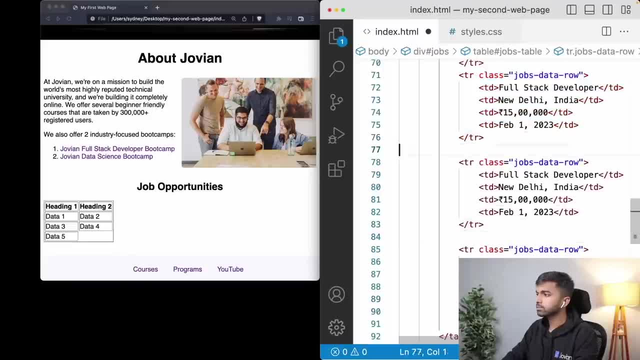 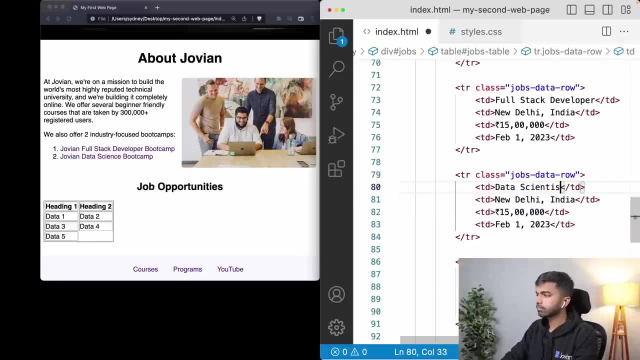 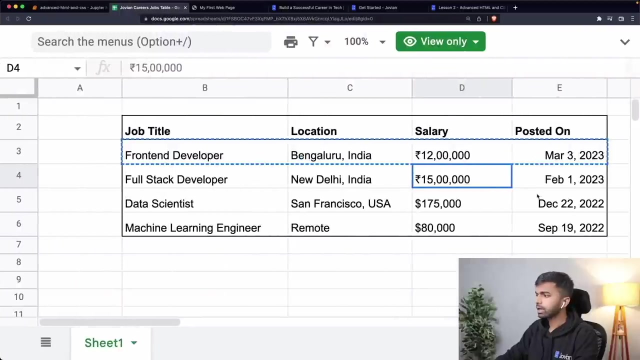 let's create a couple more copies for the next couple of rows. okay, we have a data scientist. this is in san francisco, usa, and this is, i believe, 75 000 yep, and this was posted in december 22, 20 december 22nd 2022. 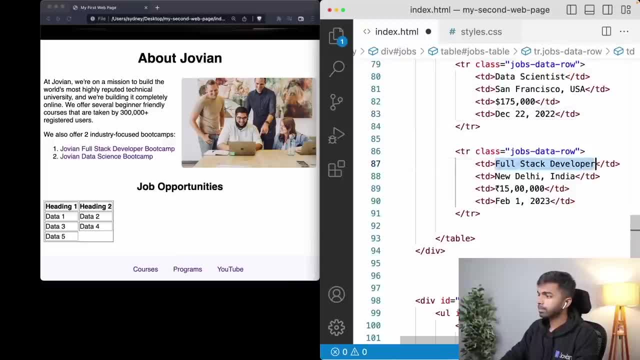 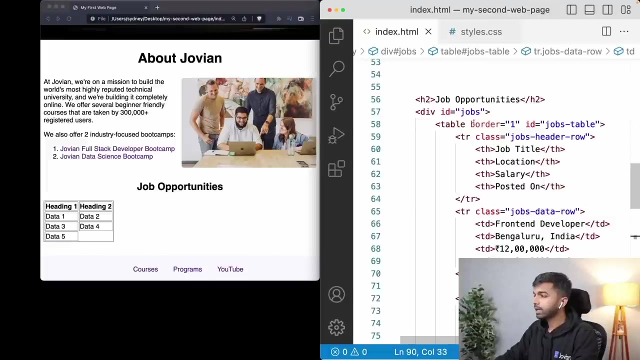 and finally, let's get that last role in here as well: ml engineer, and this one is a remote job and this one is eighty thousand dollars, and i believe this was posted on september 19th. okay, so that's our table. we have a table inside the main div and then the table has a border and the table has the id jobs. 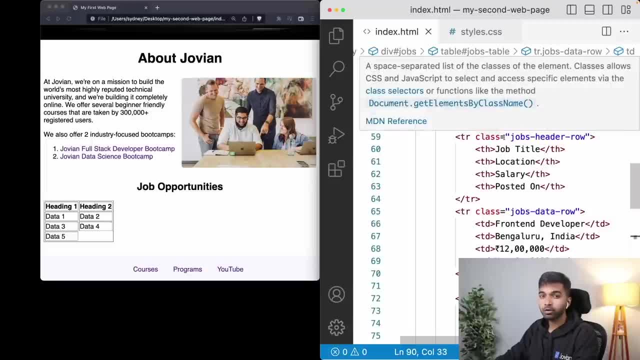 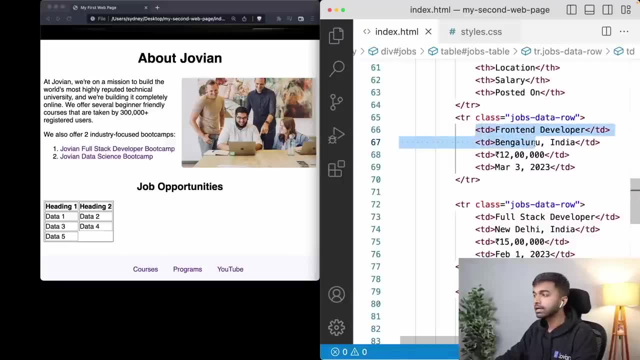 table. then we have these rows, and the first row is the jobs header row because it is for the header. we style headers separately. and then the rest of the rows are data rows and we are using tds inside instead of eh, which is what is used for the header. 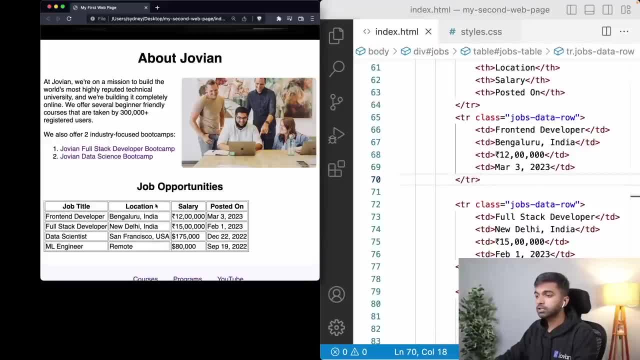 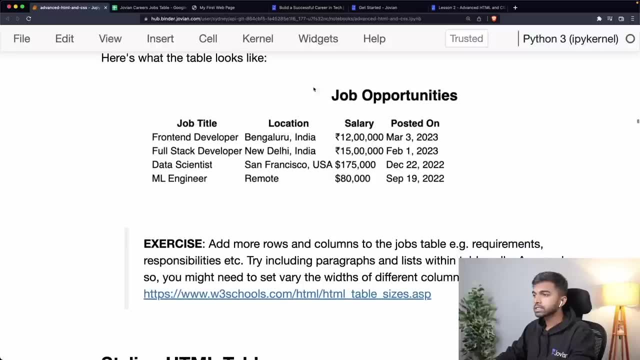 and let's save that and let's reload the page and you can see here now we have the job title, location, salary posted on and we have all the information here that we had in our spreadsheet. so this is roughly what our table looks like. we do have borders, but the borders are not very pretty. 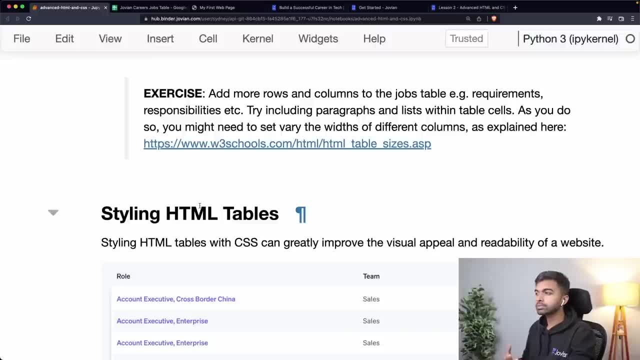 so, as an exercise, i would encourage you to try adding more columns to the jobs table, for example, requirements and responsibilities, try including paragraphs or lists within table cells and as you do so, you might need to vary, vary the widths of different columns. you might need to say that the 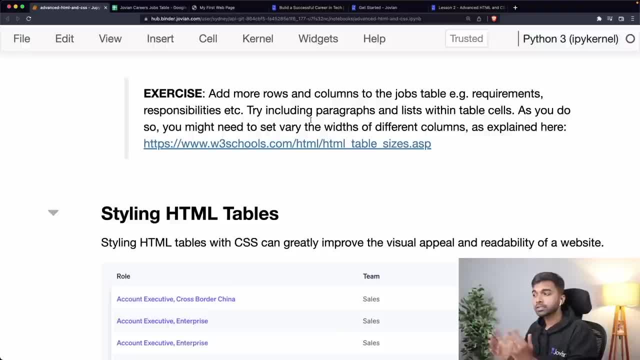 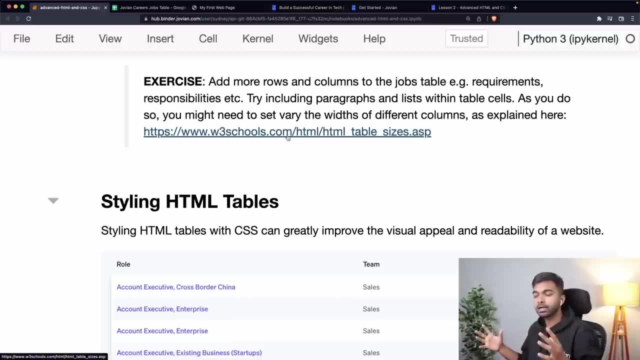 requirements column should be at least 30 percent of the table's width, and so on, and that is something that you can add by following this tutorial. so let's get started. so let's get started. sometimes, depending on the kind of data you have, you may need to vary the widths and 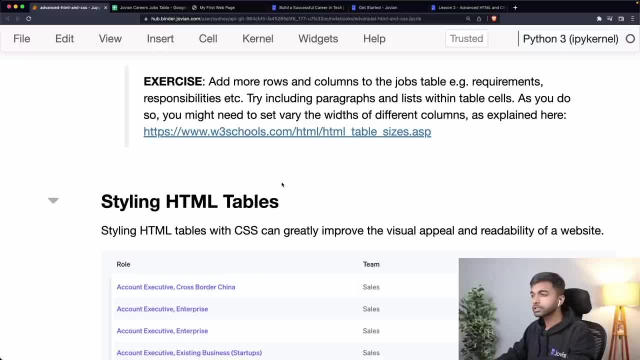 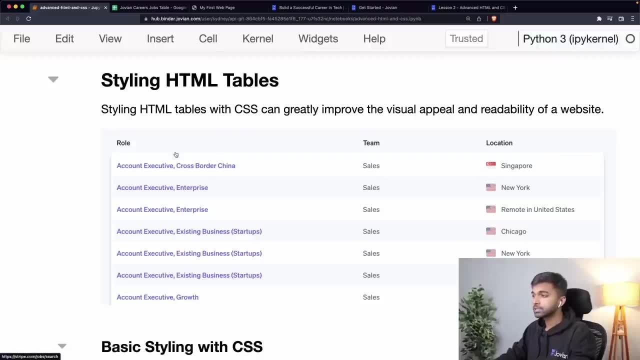 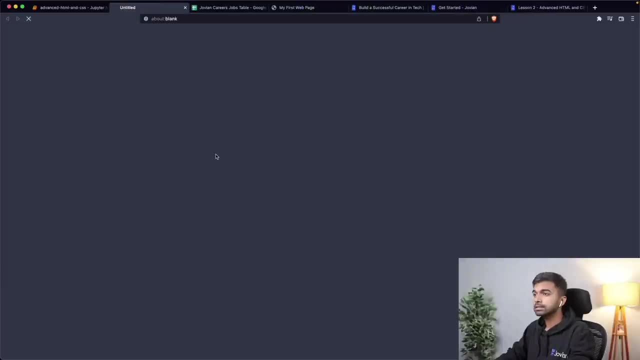 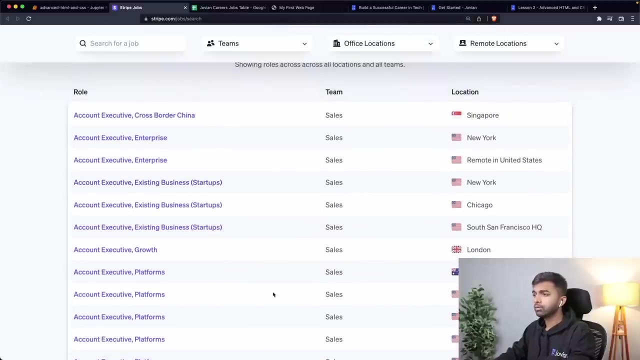 that is all something you can control using css or just using normal table attributes, but let's talk about styling html tables. styling html tables with css can greatly improve the visual appeal and the readability of a website. so here, for example, is the careers website at stripe, which is a payment processor company, and you can see that they're also using a. 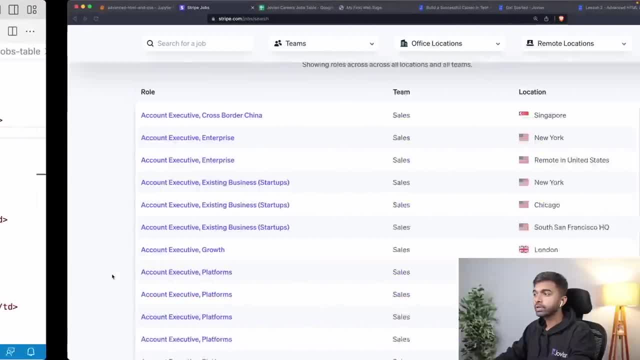 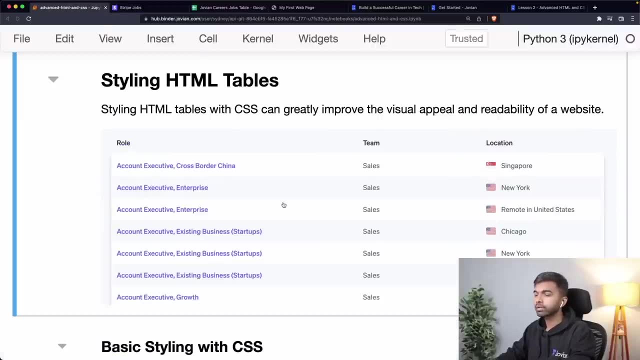 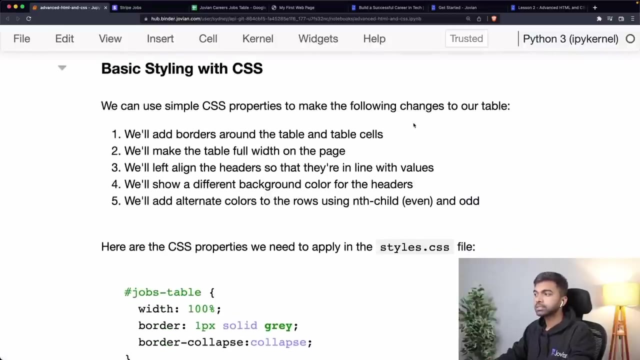 table, but their table clearly looks a lot better than our table. so let's try and make our table look a little better. not exactly like this, but we'll try and come close. so here's what we're going to do. we can use simple css properties that we already know to make some changes to our table. 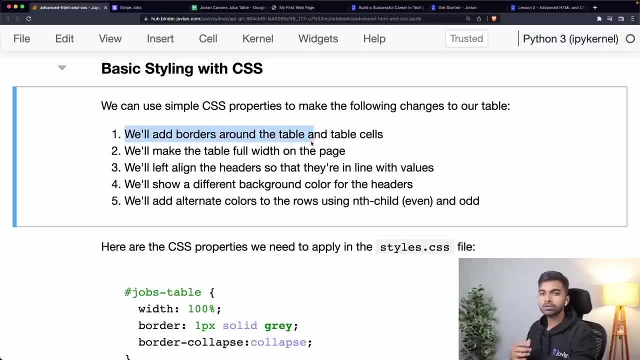 one. we'll add borders around the table and table cells using css- not using the border property or the border attribute, because css allows us to control other things like color. then we will also make the table full width on the page and then we'll align the headers we left. 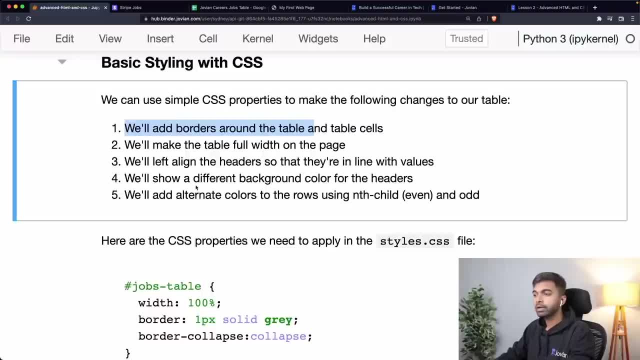 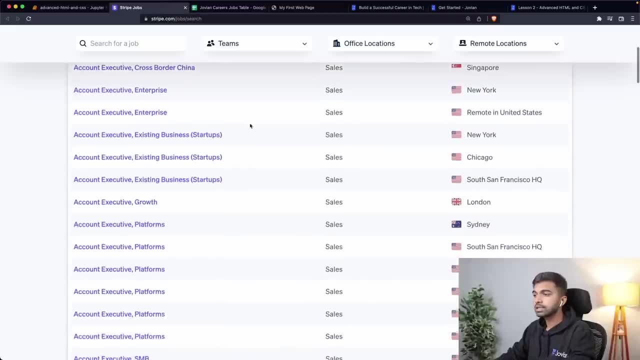 align the headers. headers are central by default. we left align them and we'll also show a different background color for headers and we'll add alternate colors to the rows. so here, for example, you can see that rows have alternate colors, so we'll add this kind of an alternate color pattern. 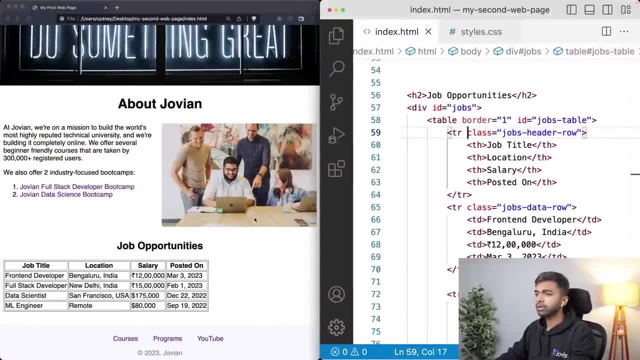 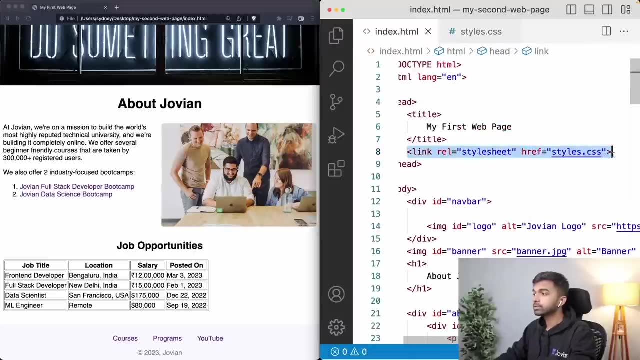 to our table as well. okay, let's try doing this step by step. the first thing i'm going to do is i'm going to add a slider to our table and i'm going to style it by putting some content into the styles dot css file, and remember that the styles dot css file is linked here. 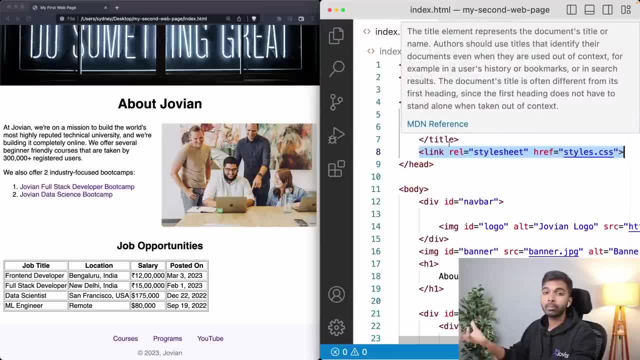 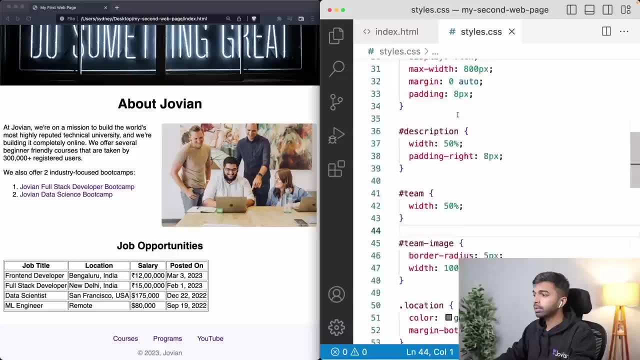 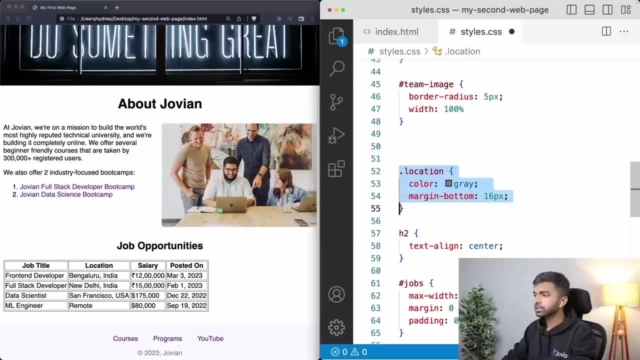 using a link tag from the head tag of the page. that is how you connect a css file to apply the styles into an html file. okay, so let me open up stylescss and i am going to come down here to: let's see this region over here. so i think we don't need this dot location. this was there in the 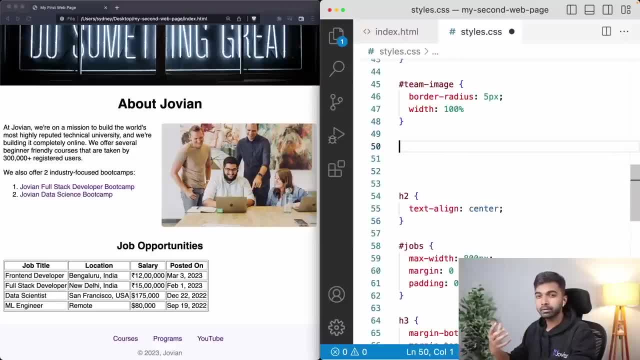 previous page we did. let's go to the next page and we're going to be doing it in a different way right now. let's model it a little bit, a little bit in each page, in each page, and then we'll make a cloud page. but we don't have location with this class anymore, So we don't need that. 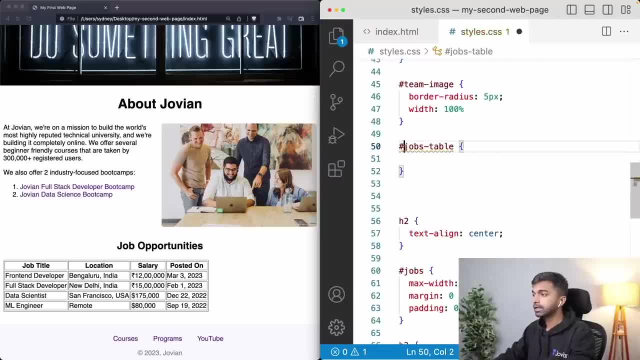 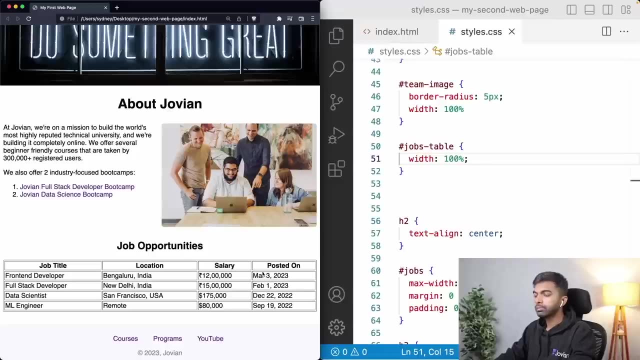 Let's put in the table, let's select the jobs table. So I'm selecting it by ID, So I'm using the hash or pound character to select the jobs table by its ID: jobs hyphen table. And let me set it to width first, 200%. So what I wanted to do is take up the entire width of 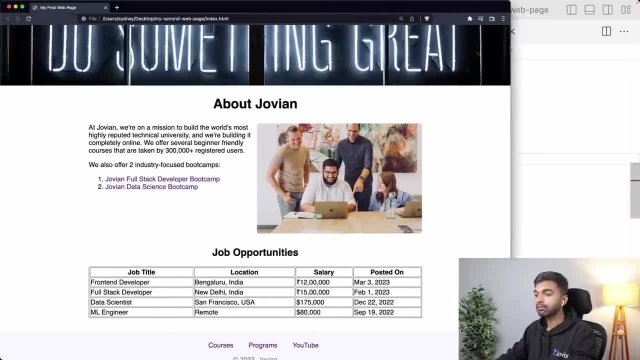 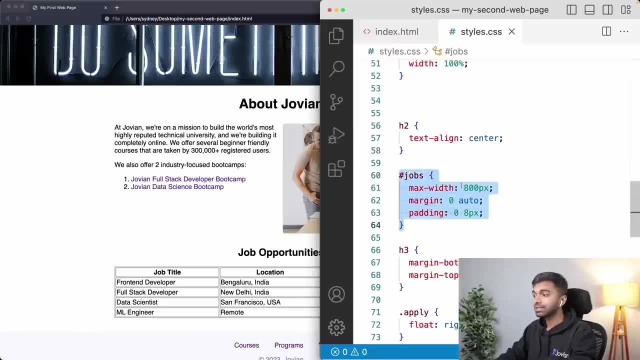 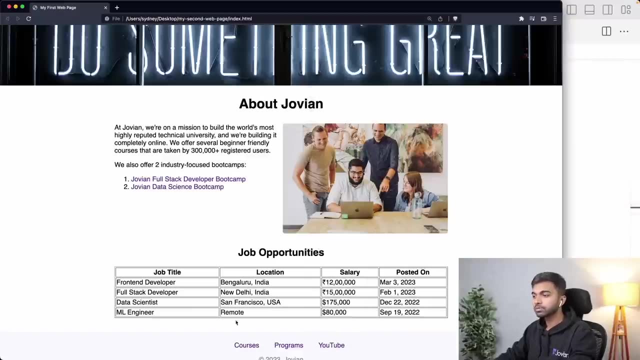 the parent div. Okay, Not the entire width of the screen, but the entire width of the parent div. You can see that we have this jobs, we have this jobs div over here, And this jobs div is set to have a max width of 800 pixels and it has a margin of zero auto. that is what centers. 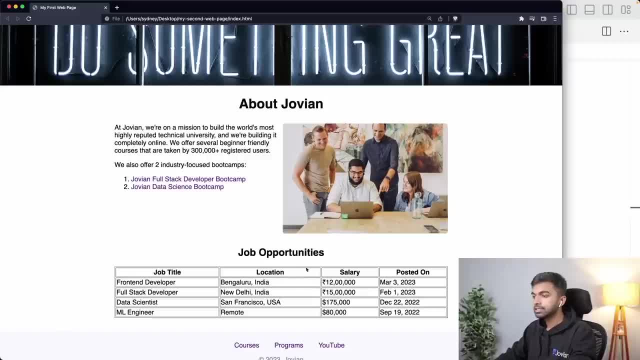 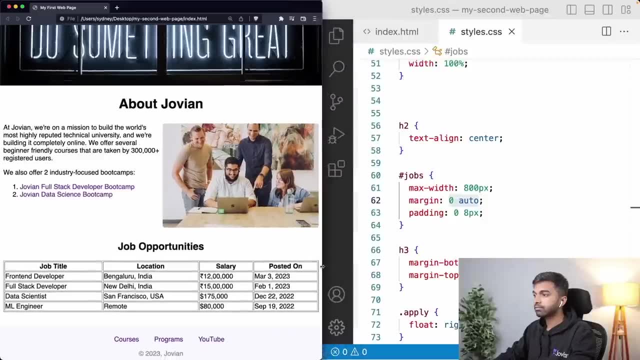 it on the page. So there's this outer jobs div And inside it we have this jobs table, which is now taking up the entire width of the parent. Okay, so that is one way to specify width. apart from pixels, you can specify it in percentages. Okay, that's great. What next? Well, 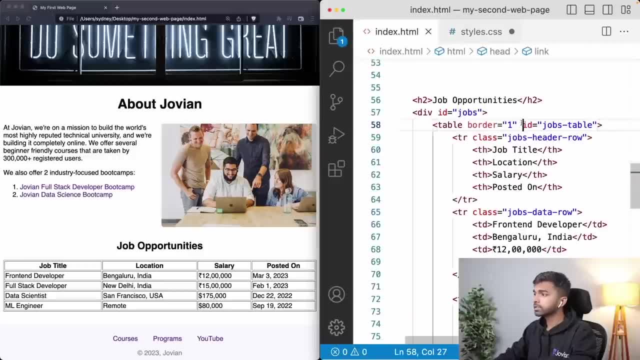 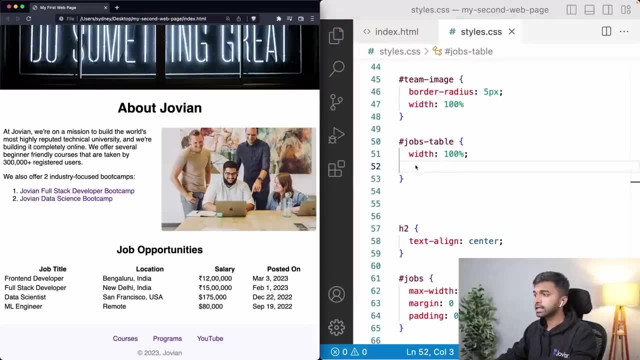 let us now add a border. So let us remove the border from here first, And let us first look at that how it looks. Okay, this is what it looks like. Let's add a border here. So border, one pixel, solid border. there are various border styles. solid means you do. 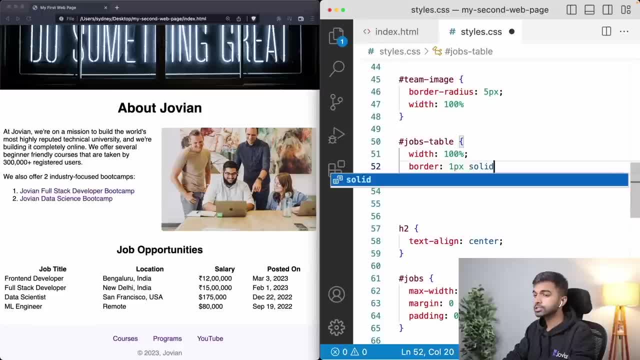 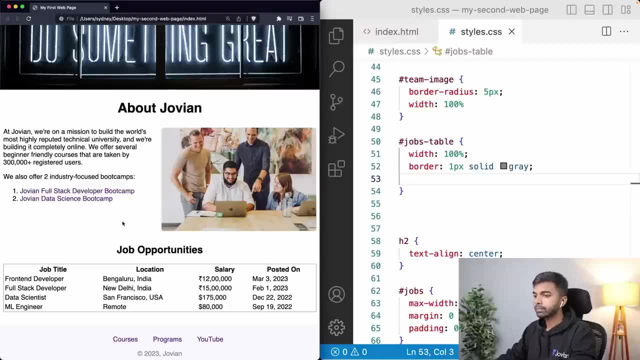 not want any dashes or anything in the border. So complete, continuous, straight line, And let's make it great, Let's not make it black. So that's the border. Let's see, Okay, okay. so now we have a border for the table. But apart from the table, we also need to add a. 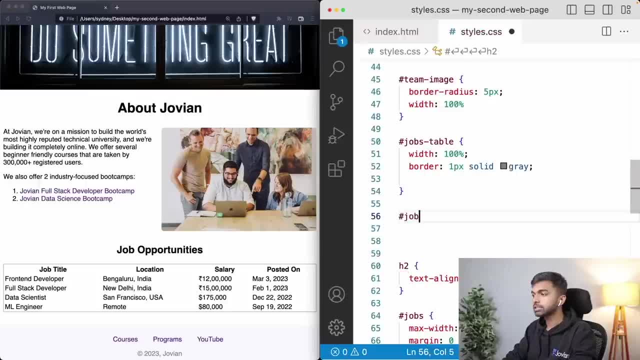 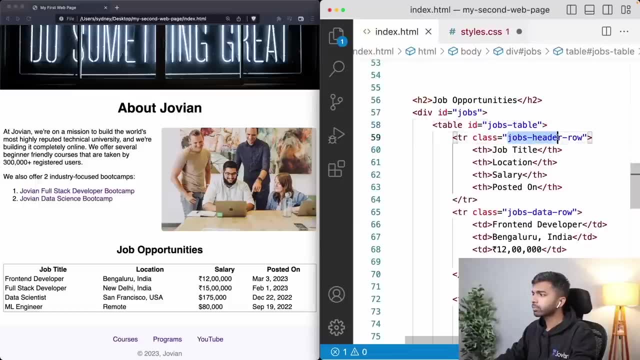 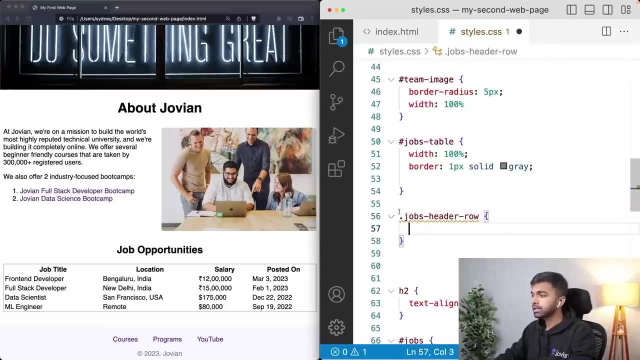 border for each cell. So I'm just going to say jobs table, Or actually I'm just going to select the cells. Let's see. So we have. we have jobs header row. So let's get the header row using jobs header row. And this time I'm using the dot selector from CSS, not the hash selector. 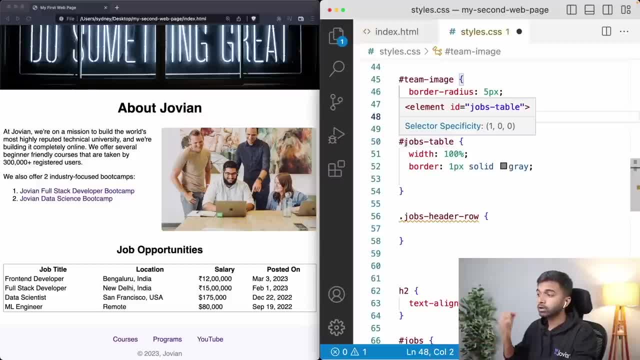 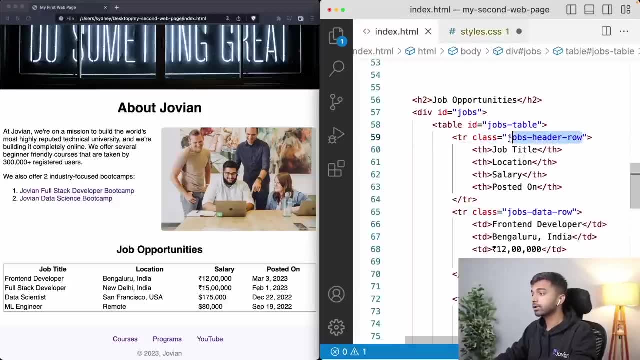 because the hash selector is used to select by ID But the dot selector is used to select by class And this T or this TR or this row here has the class jobs header row. That is why we're using the dot selector. Okay, And I am going to give. 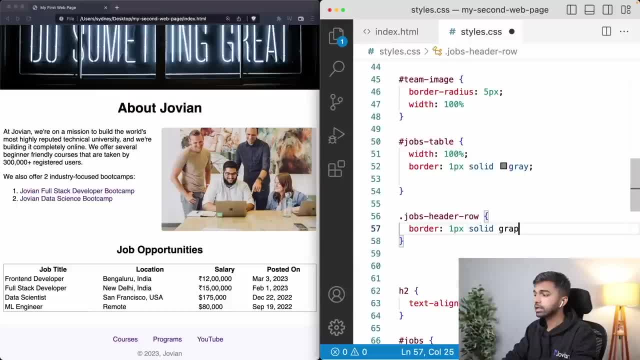 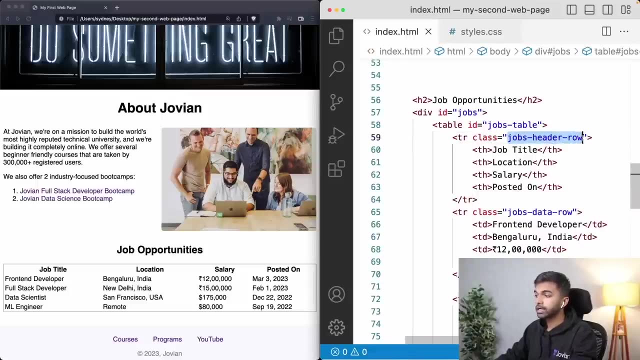 it a border as well. border one px solid gray. And oops, this is not doing it. So if you notice the class jobs header row. but what we want is a border around each cell, not around the entire row. So that is where we have to select that th cell inside the TR of the class jobs header row. 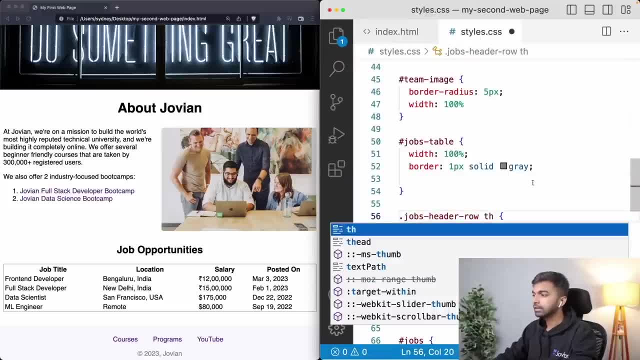 And you can do it very simply by simply writing the tag that you want to select. So now what we've done is we are saying: select using the class jobs header row. So that is going to select the row, that is going to select this row. And then we are saying inside the jobs: 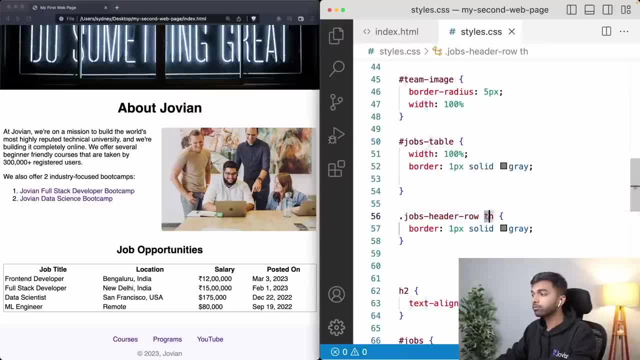 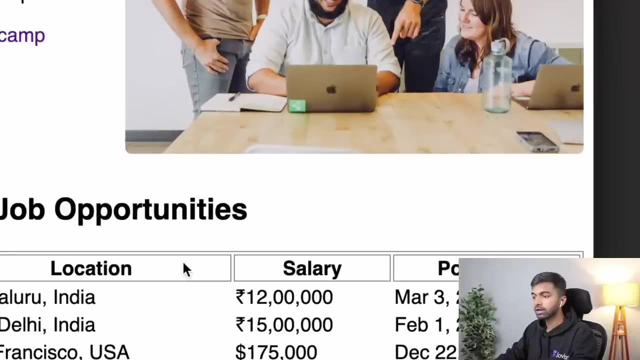 row class. inside an element with the class jobs at a row, look for a th, look for a table header cell and apply this border to it. And now, if I reload, you can see that now our table headers have these borders. Okay, I hope you can see this. our table headers now have these borders. 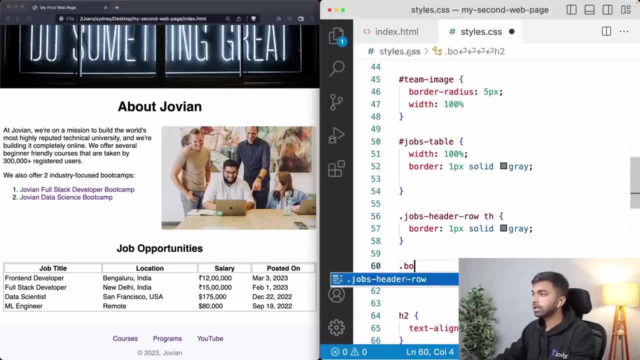 Let's also add borders to the table cells, So I'm just going to grab the data row class. So jobs data row is the class for the row containing the jobs data. And now we have the TD or the table cells over here which contain the actual data. 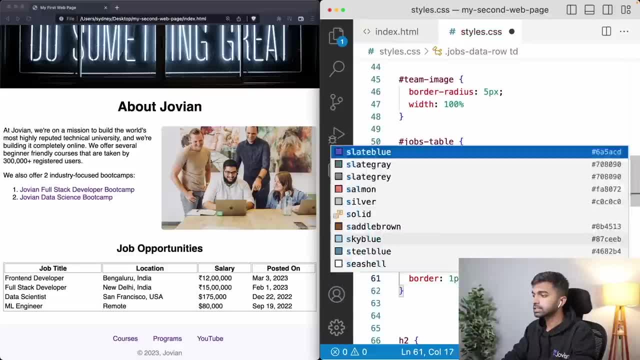 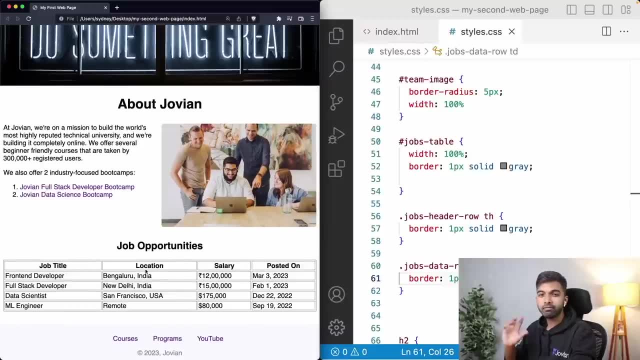 And I'm going to set border one px solid gray. Okay, and let's set that as well. So now, once again, we have borders now, But now these borders have been added using CSS, which is somewhat nicer. we have more control Now. the next thing I want to show you is how to get rid of these double. 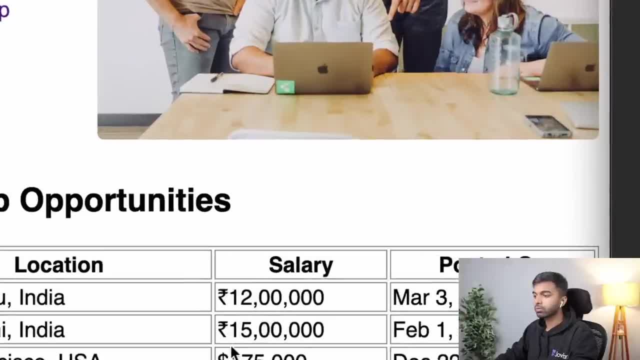 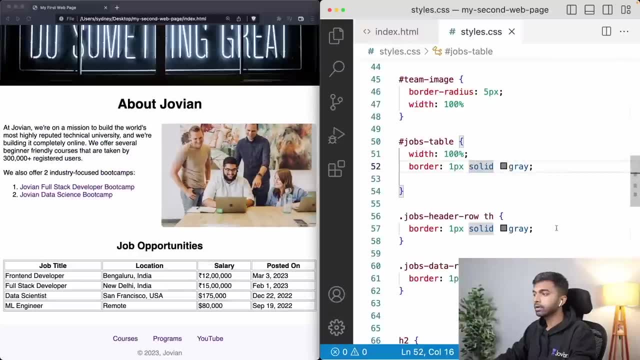 borders. you can see that we have these double borders over here, So we have the salary posted on and then we have this border around it and then another outer border around the table. The way we can do this- and this is something that you just have to look- 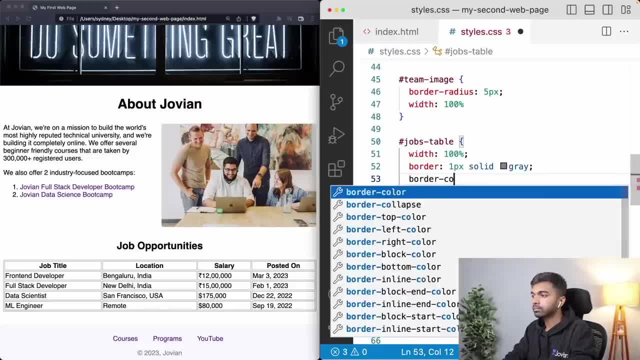 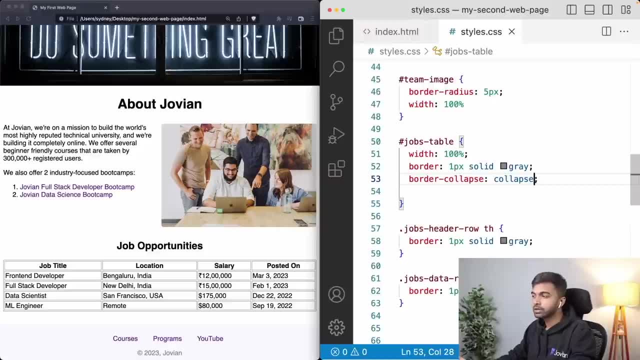 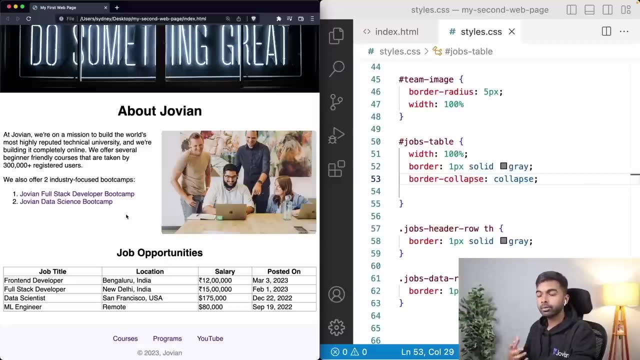 up is using the border collapse property. Okay so border collapse, collapse or you will almost always have to put this on a table if you're just styling from styling on your own. So I'm just going to put border collapse collapse And this is something that you could have looked up. you could 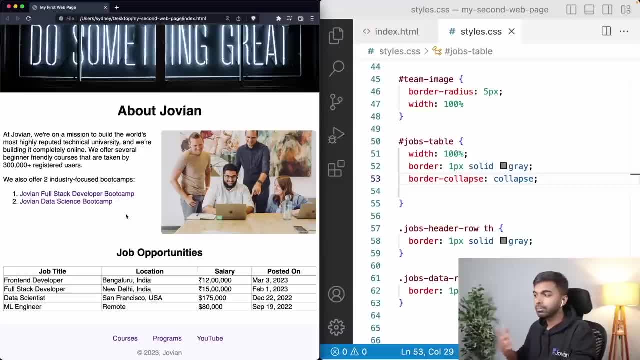 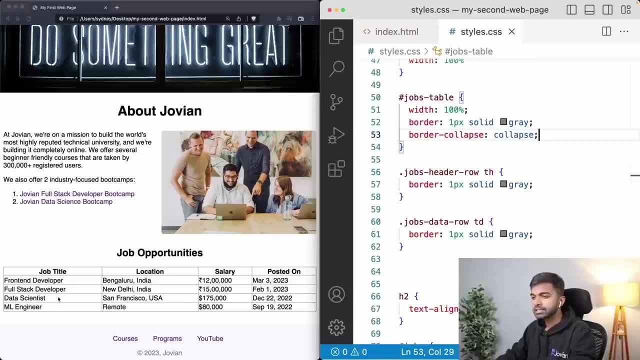 have looked up how do I get rid of the double border in a table and this is what you'll see It. But this is nice. Now I have the border collapse, or the border is looking nice. Next, Let us maybe space things out a little bit. The data is very close to the edges. 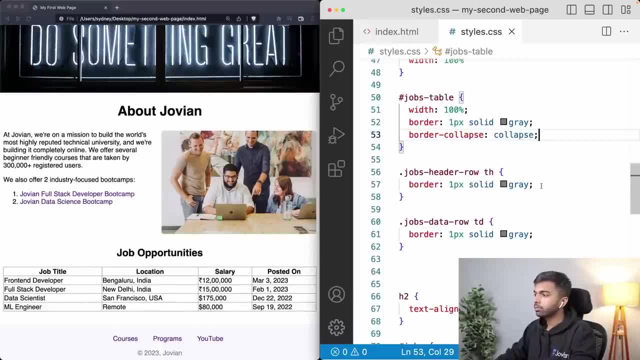 it would be nice if there was some space around it. So here's what we can do. We can go in and we can putting a put in a padding here. So let me put in a padding of eight pixels. Remember the CSS box model. 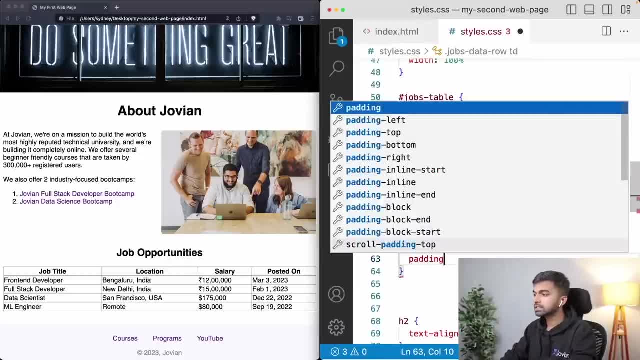 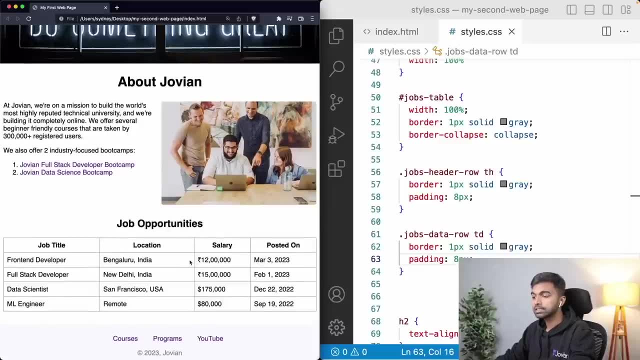 inside the border. okay, let me add a padding of 8 pixels in the data as well. so both of these will add space inside the border. so you can see, here, inside the border of a cell, we have added additional space. if we had margin, on the other hand, that space would get added outside the border. 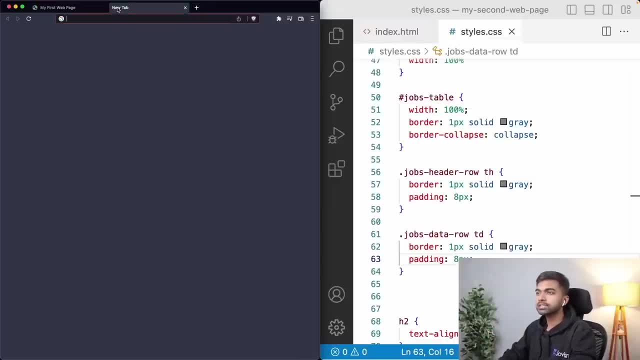 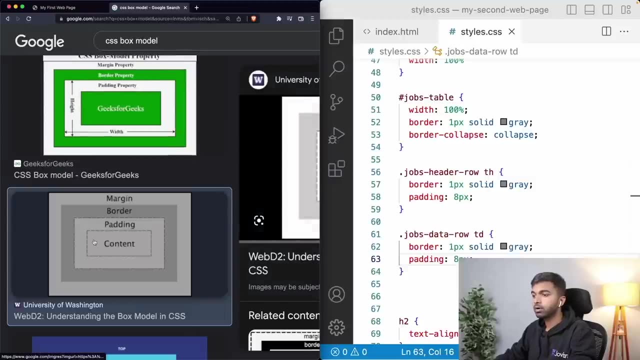 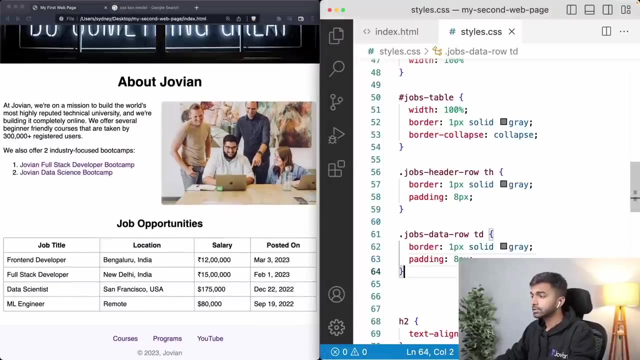 okay, so keep the css box model in mind. you can always just search online css box model whenever you are unsure how this works. okay, so we have the content, then we have the padding, then we have the border and then we have the margin outside it. all right, so this is looking pretty good. let us now 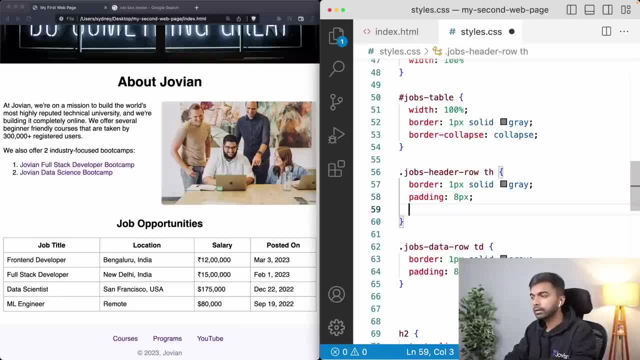 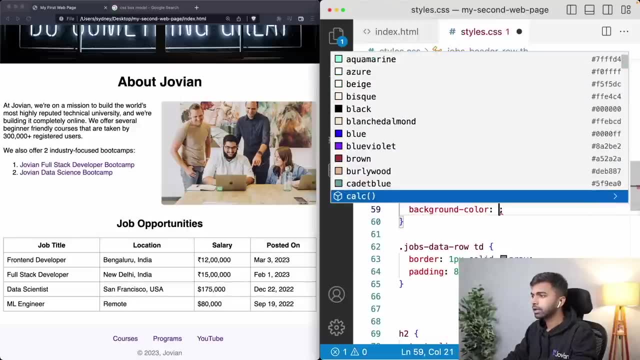 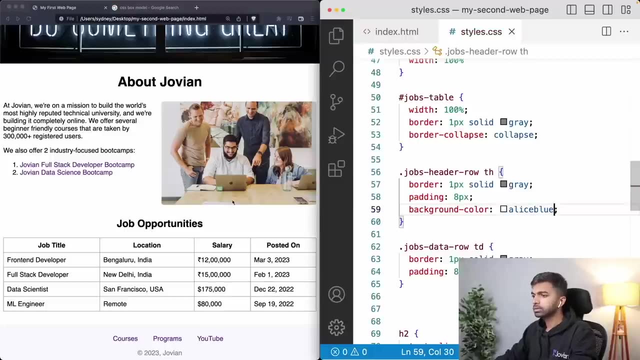 maybe add a background color to. oh yeah, let's add a background color to the header. so, background color. let's see, i am thinking of the color. let's maybe just add the color alice blue for now, one of the named colors. okay, nice, we have a nice background color for the header. i hope you. 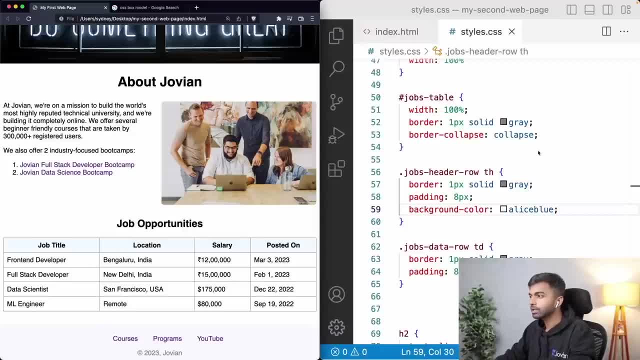 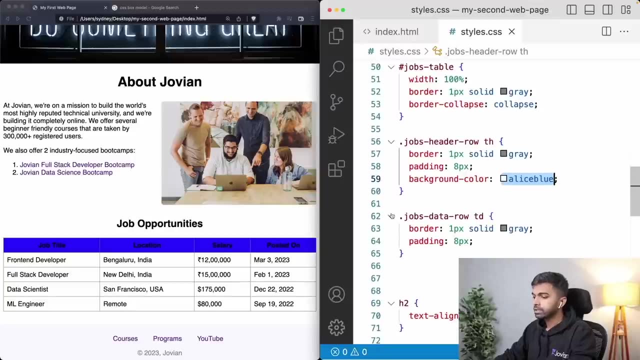 can see it. it's very light. we are not going to use very strong colors. see, what happens is, if you use a proper strong color like this, your text becomes unreadable. that is why you always want to use very muted, very light colors, and we'll talk a lot about color guidelines later down the line. okay, this is. 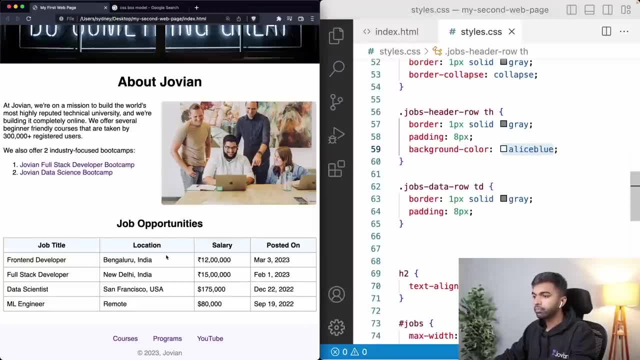 looking good. let's also add a background color now for each of these objects. we want to add a background color for alternate rows, so we don't want to add a background color for every single row, we want to add it for alternate rows, and this can be done using again. 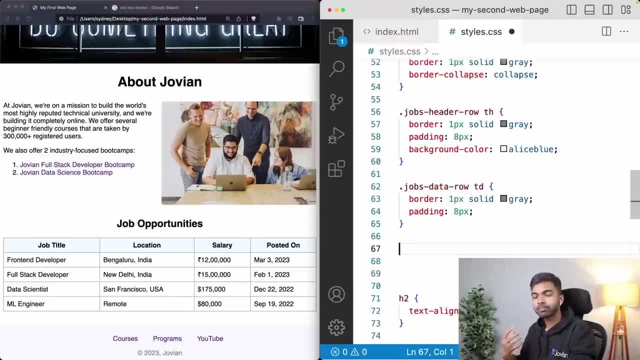 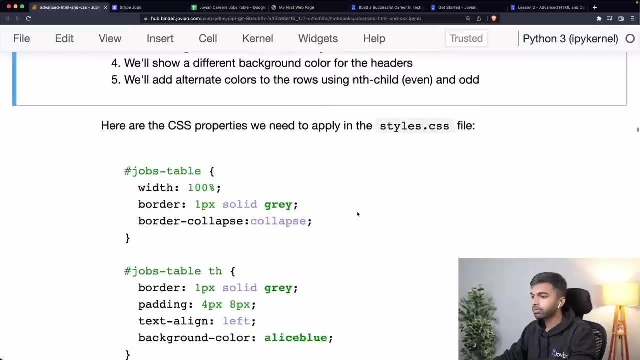 using a special property. now, this is the thing about css, that you have to look these up, look up these special properties from time to time. there's no way to remember them. i just looked it up a few hours ago. that's why i can partially remember. so you can say td and in the td, um, i'm. 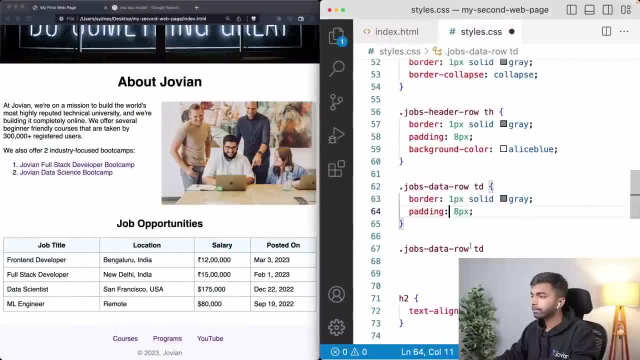 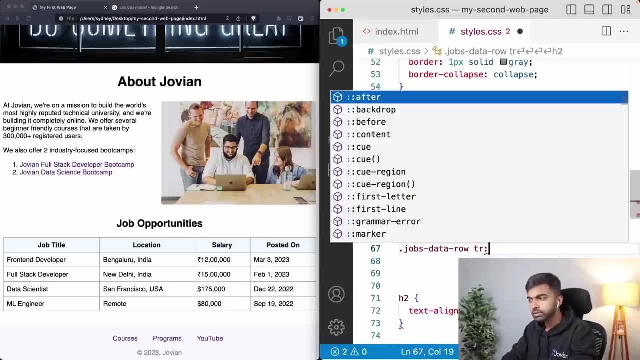 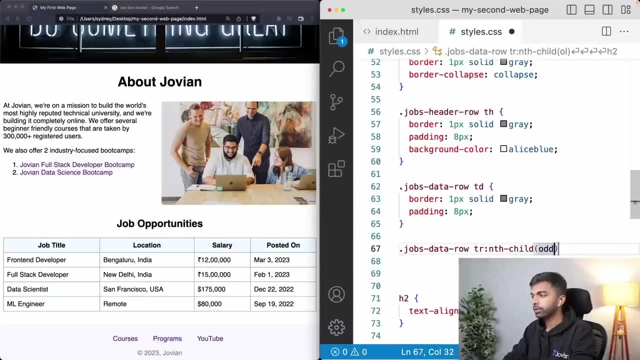 actually just going to look it up over here, or actually not in the td. i want to add this for the header row. so i want to get the rows from the table which are the nth child, where n is odd. okay, and i'll just show you what this does first, and then you will see. 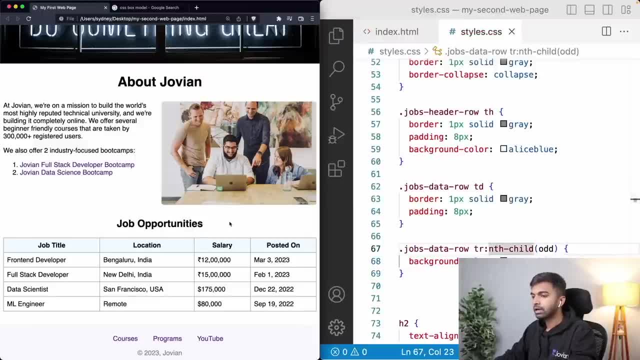 yeah, and then you will see exactly. uh, then we'll discuss how it works. okay, let me make that jobs table, yeah, so here's what we've done. we have said jobs table, so select the jobs table by id. inside the jobs table, select a tr, a row. okay, so we have the jobs table here with the id jobs table. 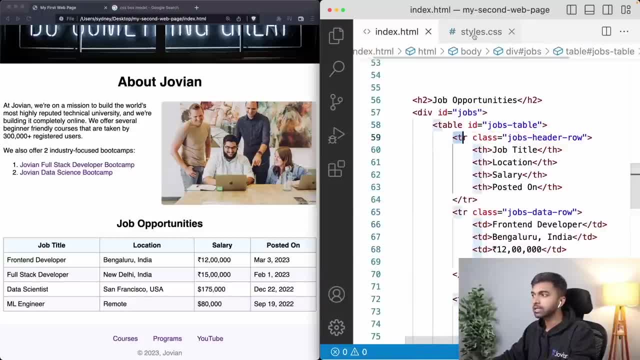 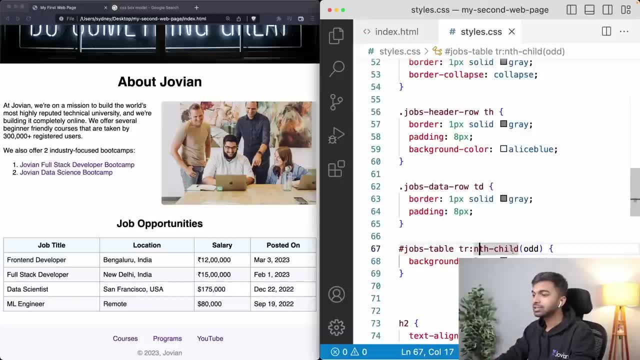 inside it. we want to select a row, so each tr represents a row. but we only want to select the rows which are: the nth child, okay, where n is odd, so all the odd rows. which selects a full stack developer row and which selects the ml engineer row, so all the odd rows get selected by putting. 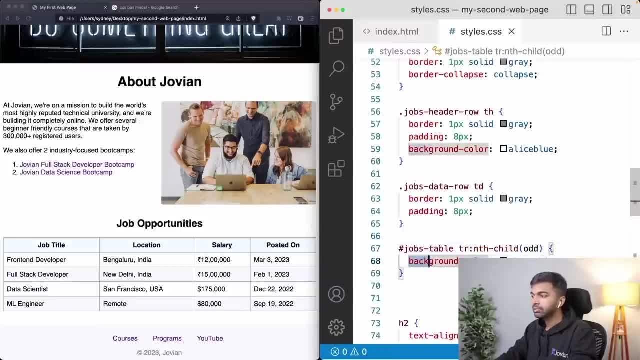 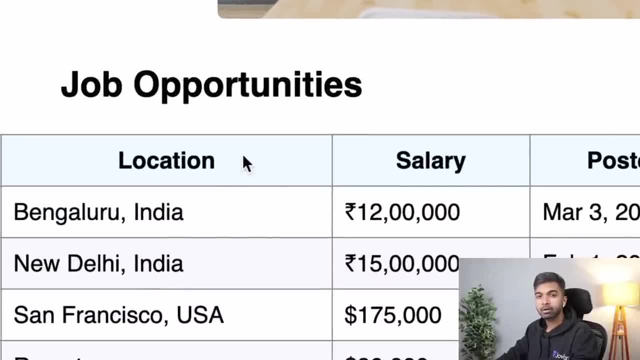 this colon, nth, child, odd, and then we are giving them the background color of ghost white. okay, again, if you see carefully, here we have, of course, a color background color for the header that we have specified. then we have this background color for the header that we have specified. then we have 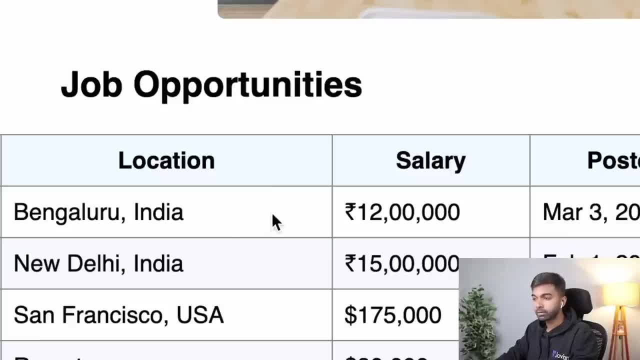 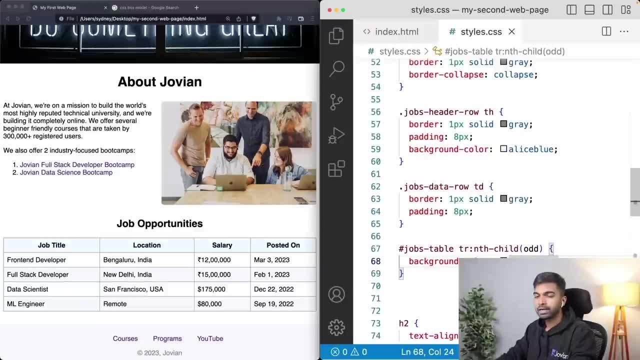 this background white color for this first row, which is row number two, technically, and then we have for the third row, new delhi, india. we have another background color- okay, it is very light, but i hope you can see it- and we've selected alternate rows using the nth child. and how do? 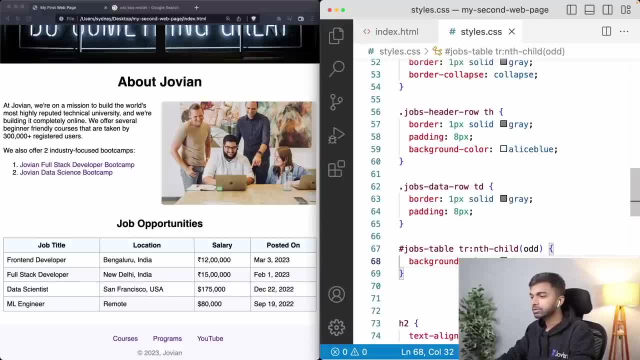 you know this well. you just have to look it up. i just look it up every time, so i don't worry about it too much. okay, great. one last thing we want to do is- maybe this is looking a bit odd, that the headers are centered, so let's maybe put the headers on the left side of the header, and then we have. 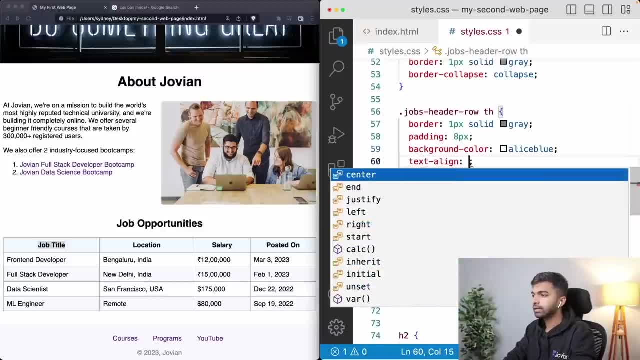 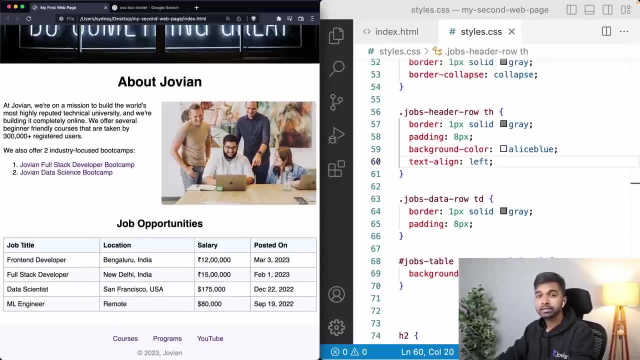 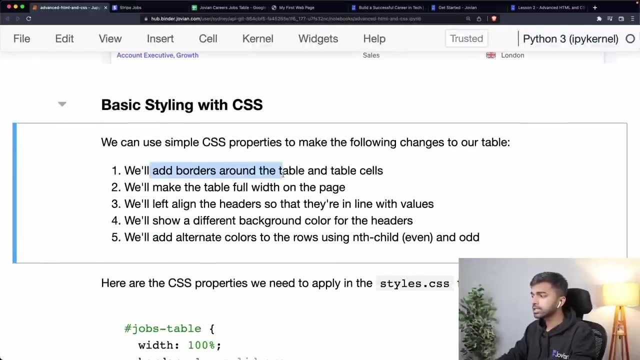 headers on the left. so i'm just going to say: text align left. okay, now the data is. now the headers are also left aligned, all right, so i think we've, with that, we've implemented everything that we set out to implement. we added borders around the table. 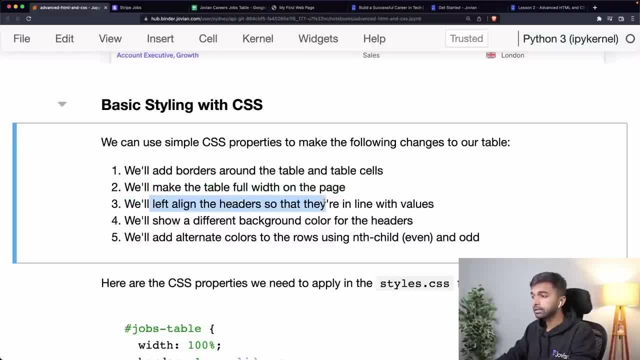 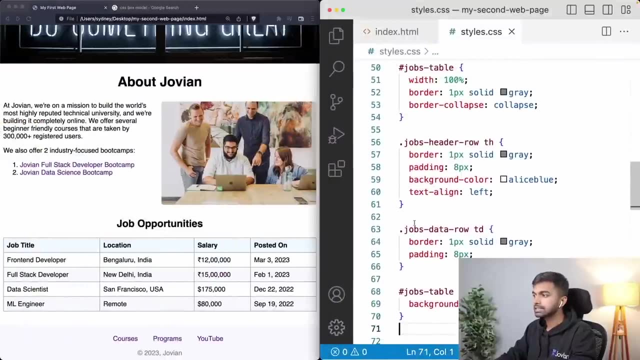 we made the table full width. we left align the headers. we are showing a different background color for the headers. we are using alice blue and we are using alternate colors for the rows. using the nth child: using the nth child- odd property: okay, so that is the css that we need. 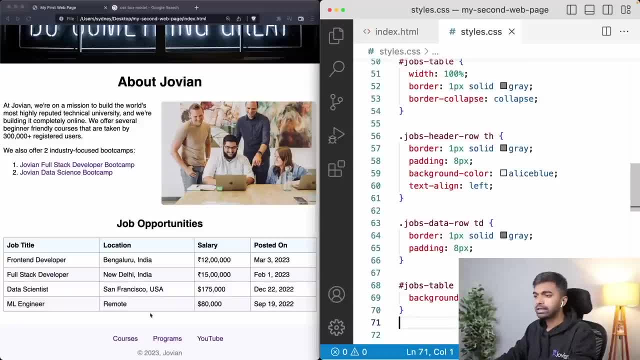 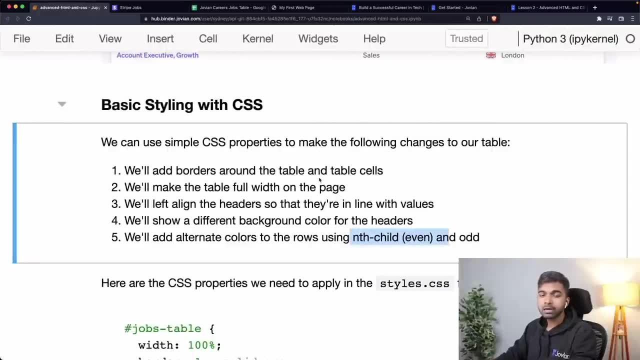 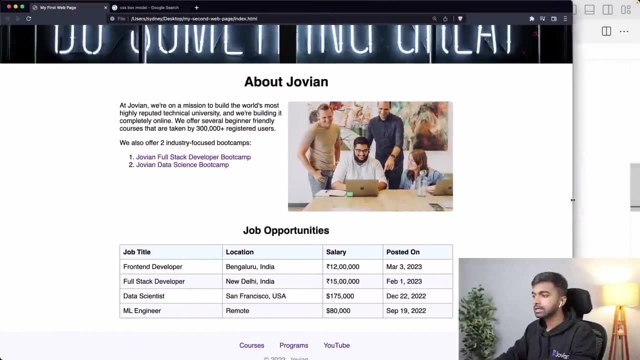 to style our table. not a lot, it's about 10, 12 lines, but it look. it makes a table look rather nice, i would think. okay, great. so that is how you style tables with css. and you can also verify, if i resize this, that the table remains in the centered and it occupies the full width of the parent. 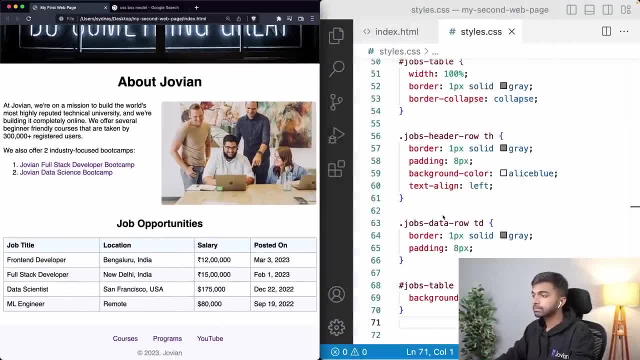 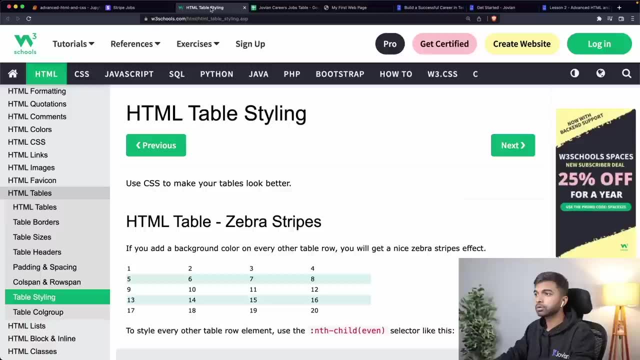 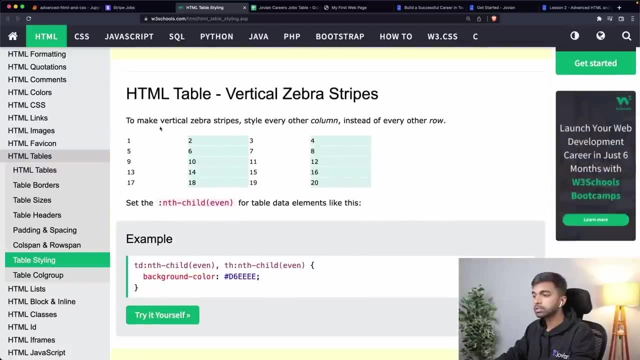 component. okay, so that's tables. now i would encourage you to maybe also learn a little more about styling of the rows and columns. so there is this tutorial on html table styling. you can have these zebra stripes, which is what we've implemented, or you can also stripe. you can also have colors for the different. 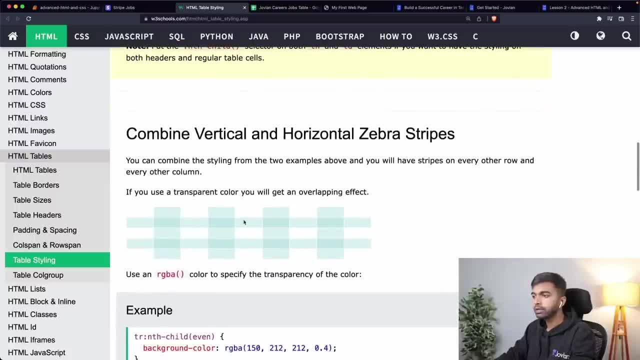 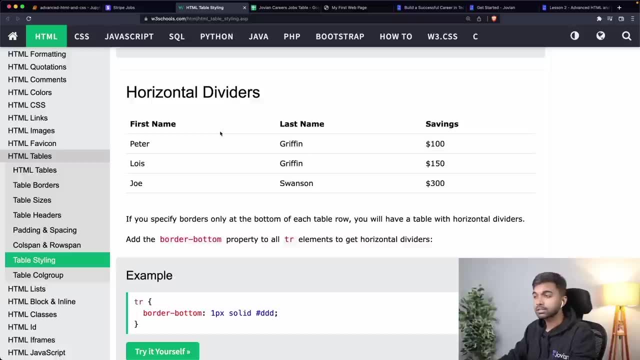 columns, if you want, again using nth child, and you can also combine vertical and horizontal stripes. so you have a lot of different ways in which you can combine. of course, you can do tables. you can have tables without borders. so one change for example we might make is we may not want the 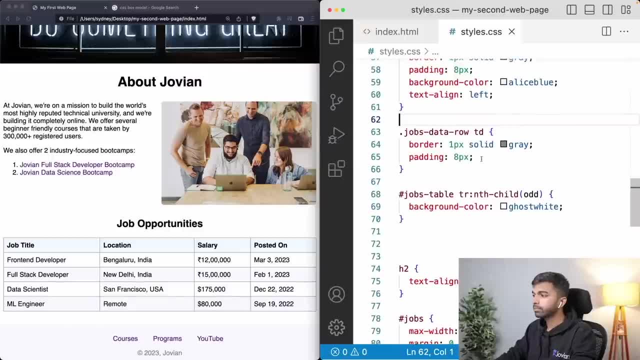 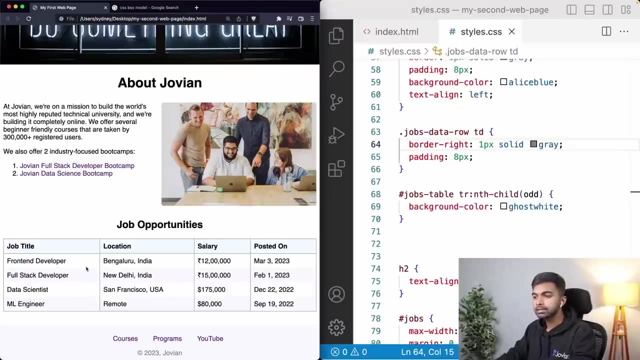 borders between the inner rows, so we can come in here and we can say that for the td, for these data cells, we don't want a border bottom, we just want a border right. okay, and what that's going to do is that's going to remove this border bottom, because we already have alternating colors. 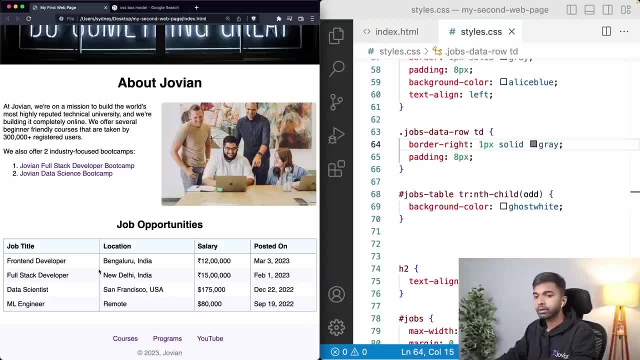 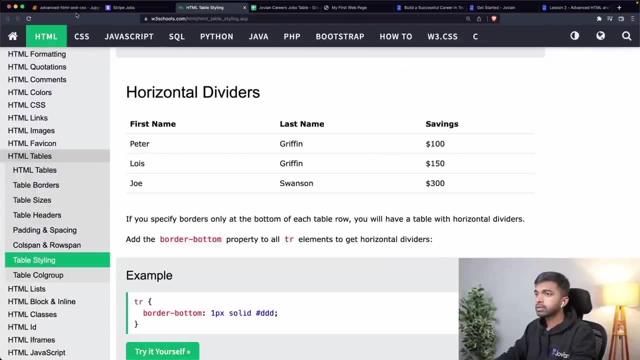 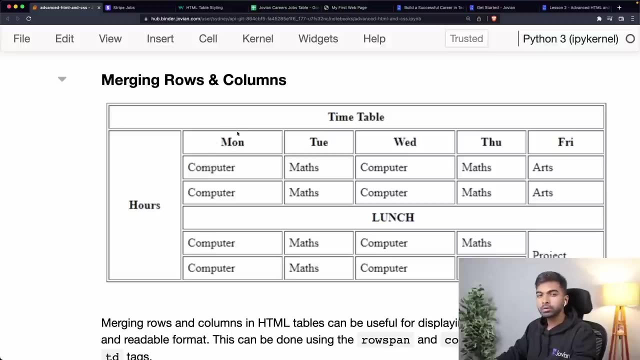 and that's just going to keep this border on the right. all right, um, yeah, so that is how you style tables in css. so, moving right along, we'll also talk a little bit about merging rows and columns of data in tables. now you can use, you can create all sorts of interesting tables. 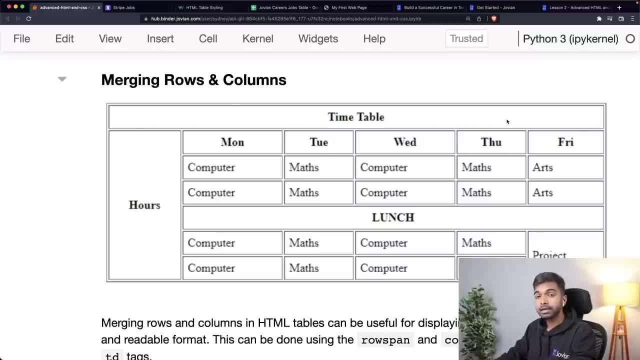 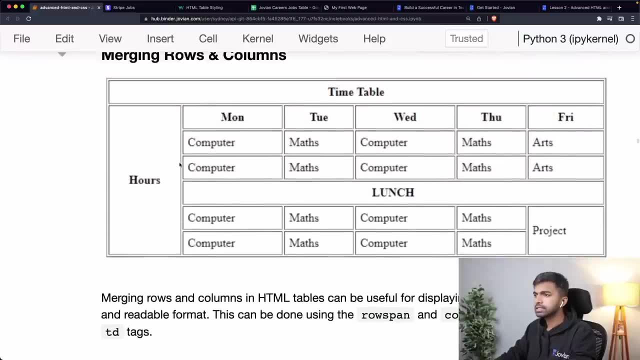 in html. what you can do is you can merge a bunch of data cells to look like a single cell, either vertically or horizontally. so what would be nice for us is to maybe try that with one of the columns here. so let's do this. let's get the location column. 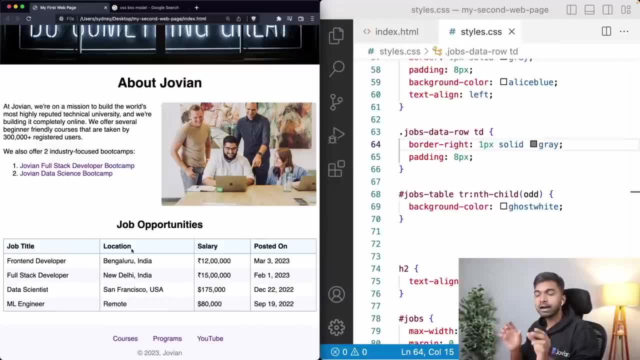 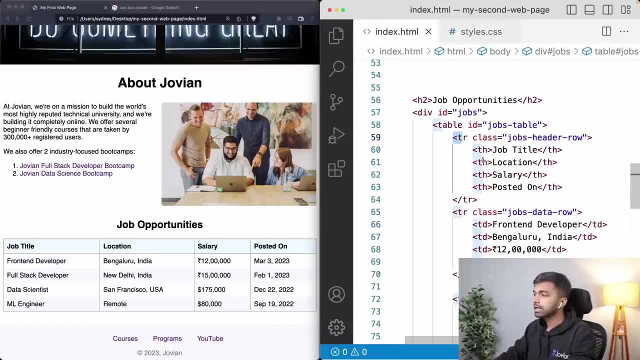 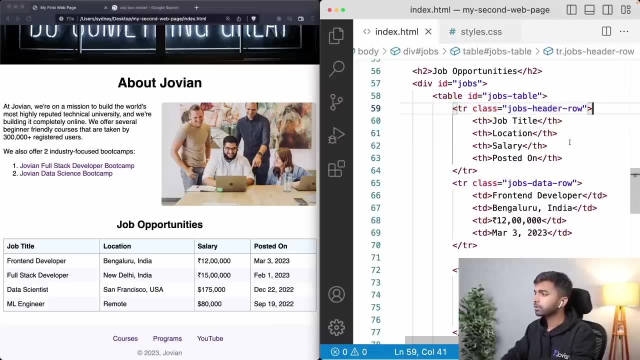 and let's have the location column split into two columns: city and country. okay, so here's how i'm going to do it. i'm going to have sub columns under location called city and country. let's come back here into the table definition and we have this first row. we have this first row. 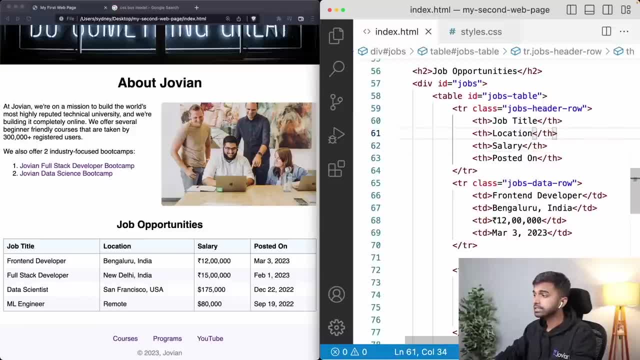 and this first row now contains a location, so that's great. let me add a second header row. so let's add tr. and here again i'm going to add: let me keep that class here as well. okay, now here i'm going to add a couple of headers. one is called city and the second is called: 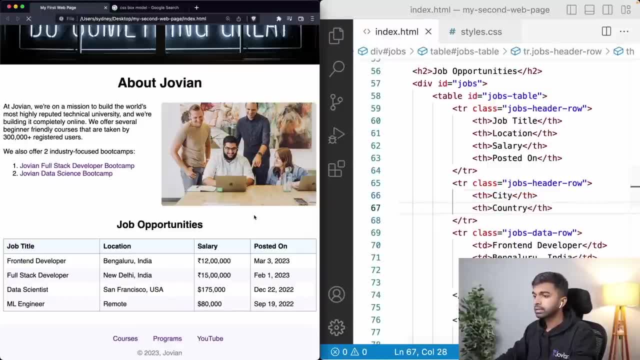 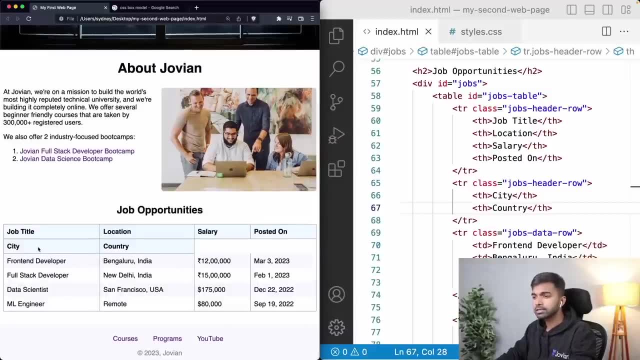 country. all right, and what does that do? well, as you might expect that, add the second row of headers. but now, in this case, the second row of headers says city and country, below job title and location. that's not what we want. what we want is to show me to make this show up under location. 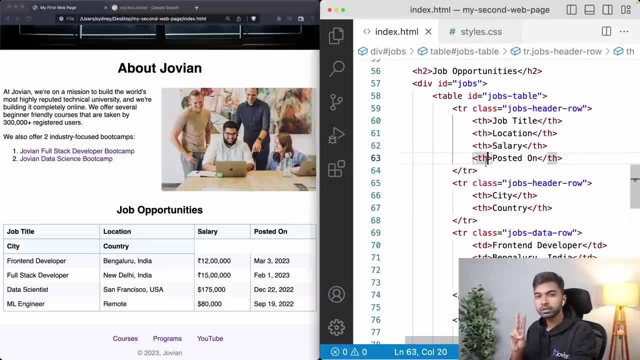 itself. so here i'm going to use two special attributes. the first is called call span or row span. okay, so we want the job title to actually span two rows, so row span equals two, and now what this does is the job title. the job title header is now taking up two rows of data. okay, we've simply 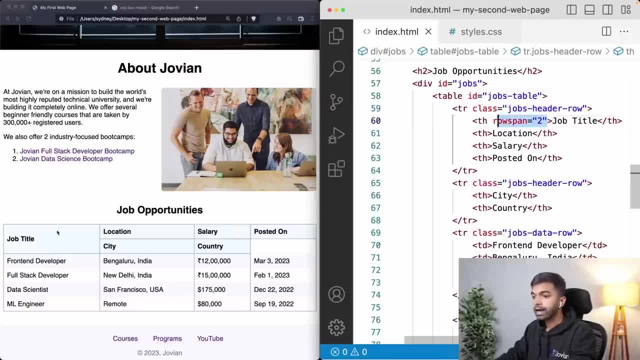 added the property row span equal to two the attribute, and that ensures that job title take up two rows of data, whereas location salary posted on are still taking up only one row of data. now we want the location to take up two columns so that city and country show up under location. 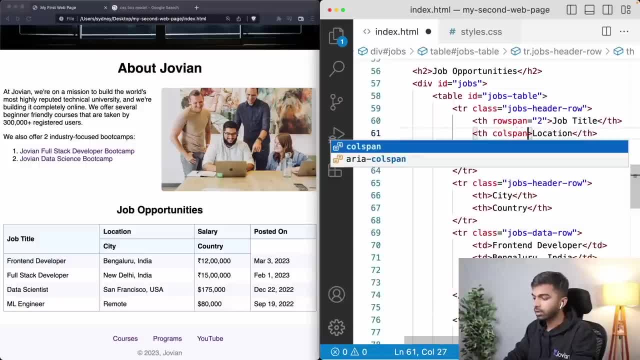 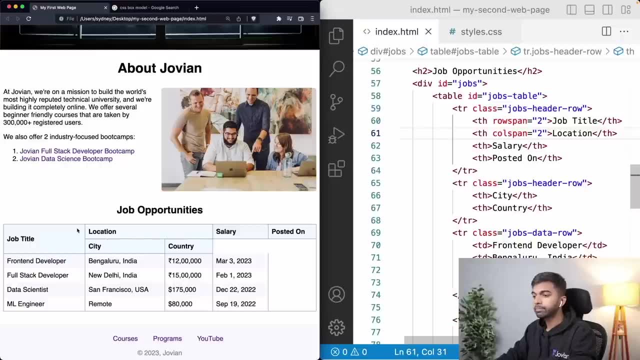 so we can add a call span and we can say: call span equal to two for location and let's reload that. and now you see that the location cell takes up two columns. so that's why the and country headers show up under location, because each of them take up only one column. 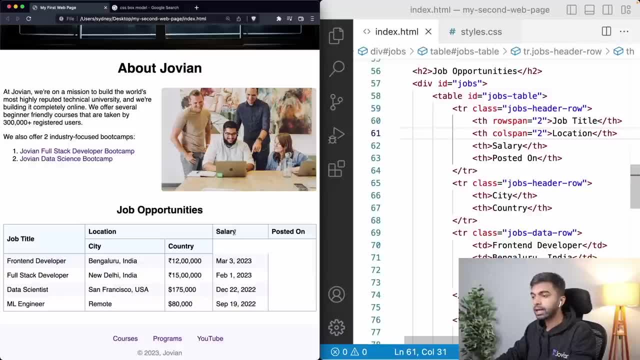 each. And now let's go ahead and finish this heading by actually giving row span of two to salary and posted on as well. So let's set row span equal to two for salary and let us set row span equal to two for posted on. Okay, So now we have the job title which 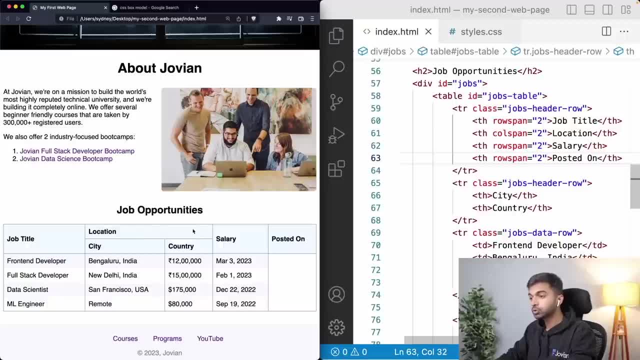 spans two columns, Then we have the location, which spans two rows. So now we have the job title, which spans two rows, Then we have the location, which spans two columns, but only one row, Then we have the salary, which spans two rows, And then we have posted on. 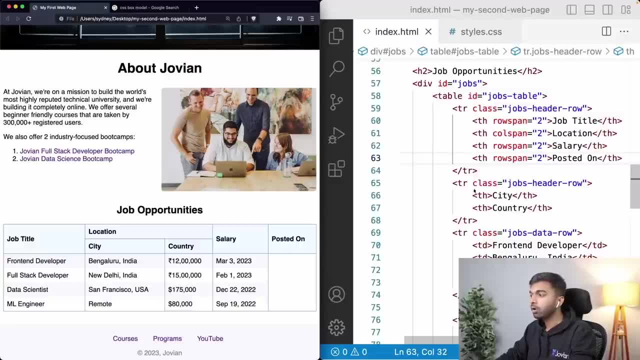 which spans two rows. However, we have now also added the second row in which we have the city and country, both of which only span one row and one column, And because we have these other values spanning two rows, they automatically get adjusted. 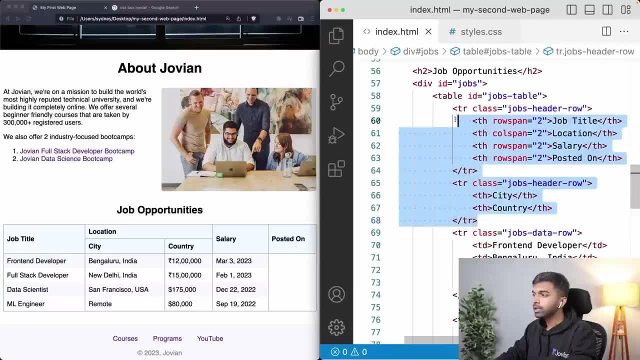 It under location. Okay, So this can be complicated at first. You're not going to get it just by watching, So practice it by watching the video, rewatching the video and typing it out step by step, And it'll start to make a lot of sense. Okay, Now finally, let's. 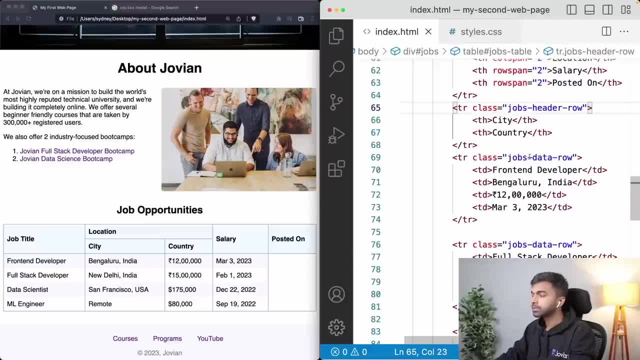 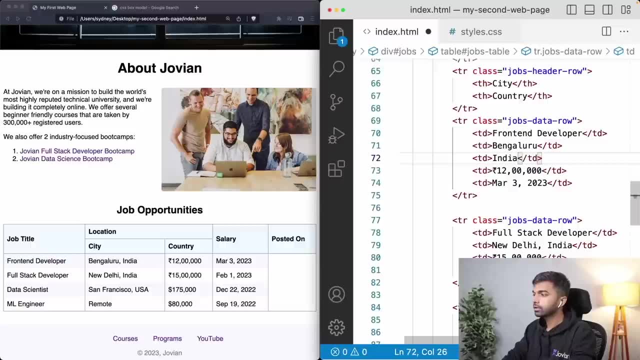 also split up the data. right now You can see that the data is a bit messed up, So let us split up the country and city for the data. So I'm going to come into the first row here, first data row, and add another column. 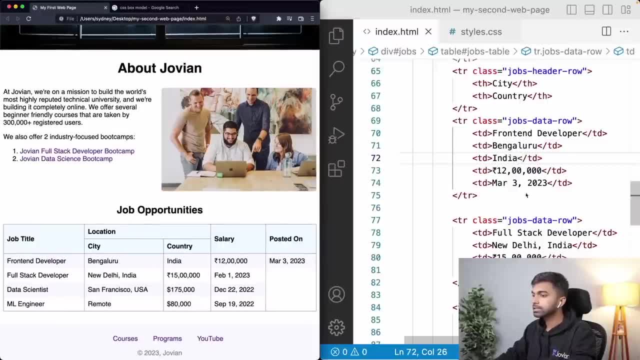 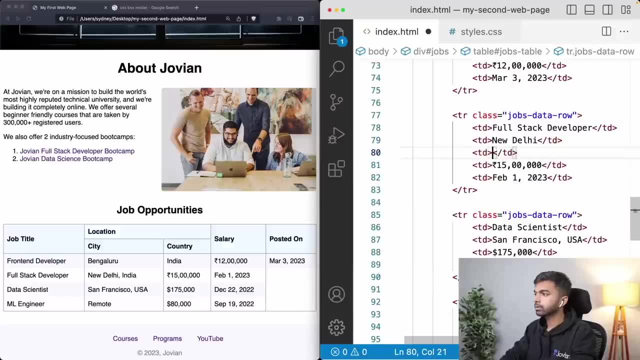 So now we have Bengaluru. India is the country and a city and country. Let's do that for new Delhi, India as well. So let's come in and add India. Okay, That's good. Let's do this for San Francisco USA. 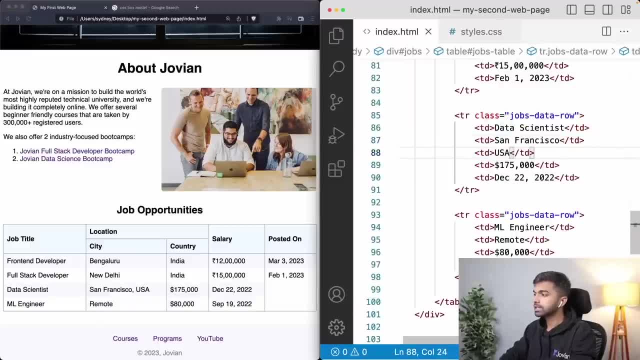 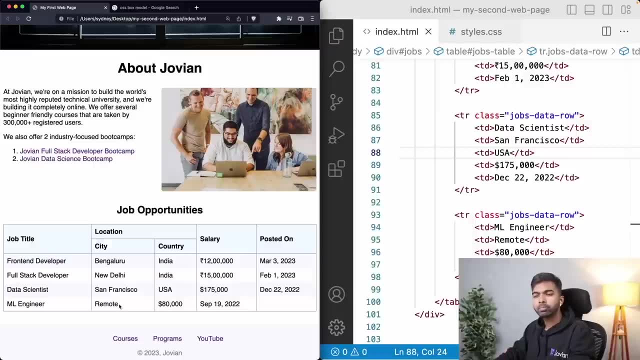 as well. Again, let's extract out USA and put it in a separate table cell. All right, So now we have Bengaluru, India. New Delhi, India, San Francisco, USA. Now, remote creates a problem for us because it's neither a city nor a country. So how about Bengaluru India? 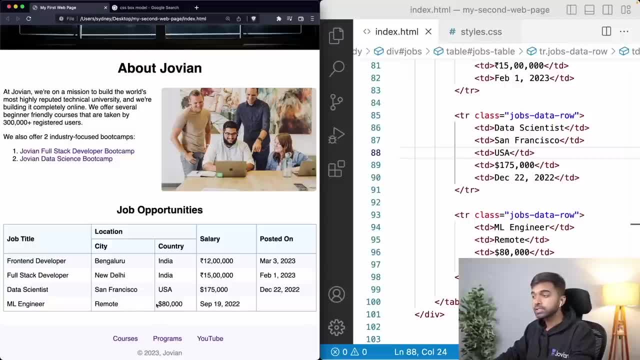 New Delhi, USA. How about we expand remote to take up two cells? So let us simply come in here and let us sell call span equal to two for remote And let's reload that. And now suddenly you can see that we have the job title and then we have the location and 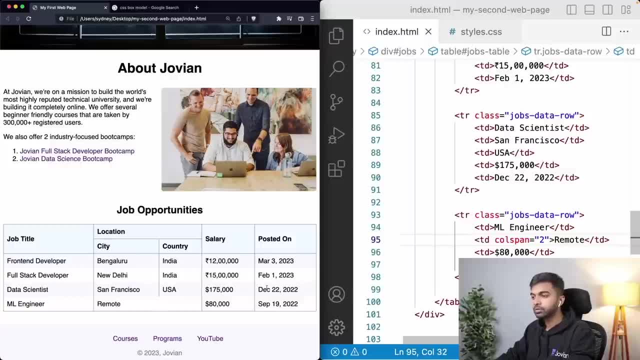 under location. we have city and country and then we have the salary and posted on, And, of course, city and country are split properly, except in the case where it is remote, where it is just a single cell. Okay, So this is how you create a more complex table: by 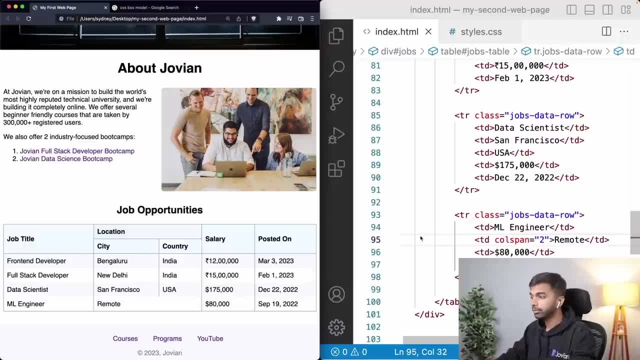 merging rows and columns using the row span and call span attributes. Now that we have this slightly more complex table, I think it might be better to maybe bring these headings back into the center. I'm just going to go in here and I'm going to remove this text. 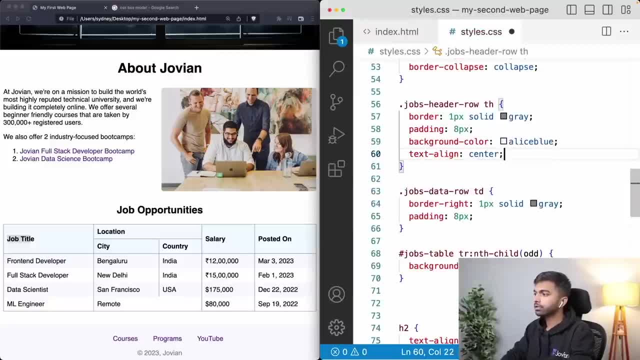 align left or I'm just going to put in text: align center for the headings. So under the jobs header row for the TH, which is the header cells, I'm going to center the headings. So I've centered the headings right here, Perfect. 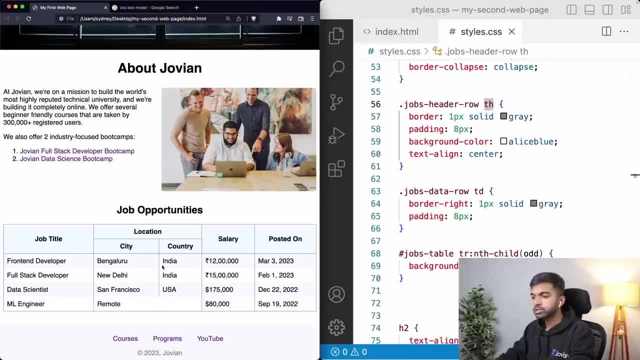 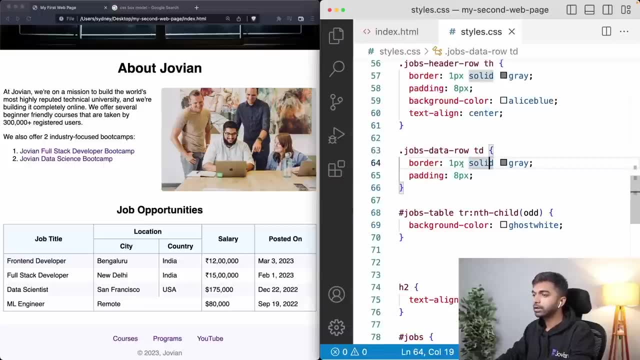 And I think I'm also going to bring back the separators, because here this line ends abruptly. So I'm just going to come in here and change the border right for the TD or the data cell to border, so that the border shows up on all sides, not just on the right. Okay, So now. 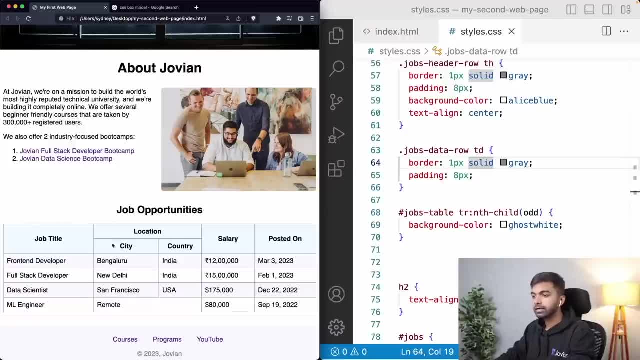 this is our job opportunities table Now. it contains the job title, It contains the location split by city and country, It contains a salary and it contains a poster on information as well. Okay, So now our table is looking very nice. We have simply added some rows and columns. 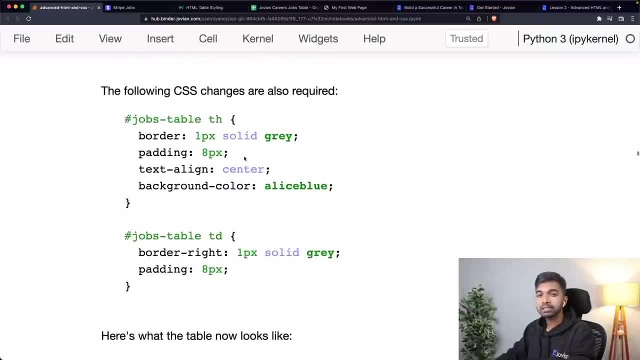 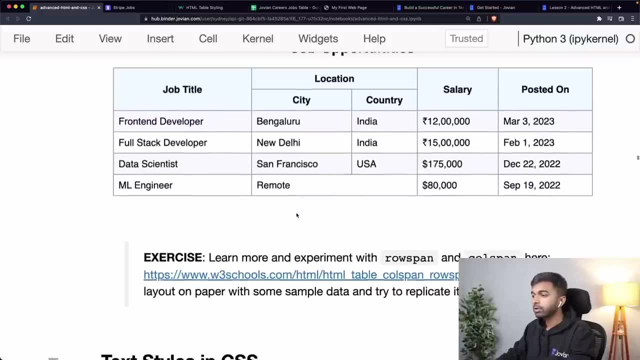 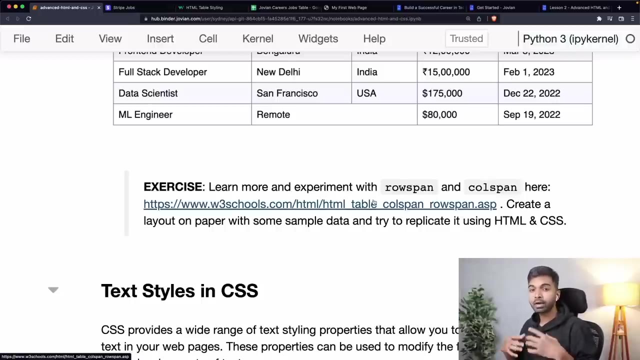 span and call span properties, and we've added some, updated some CSS to make it look something like this- exactly what we are looking for. Now you can again check out this resource to experiment with the row span and call span property, to become familiar with CSS and HTML. 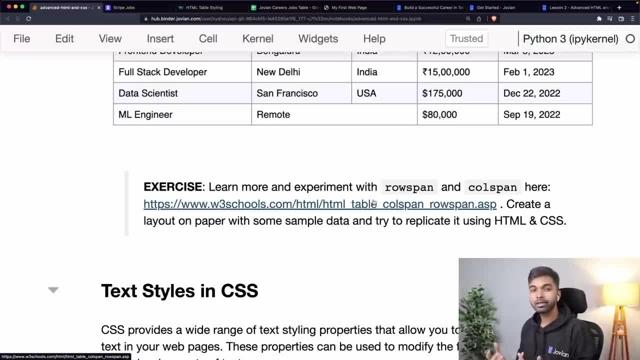 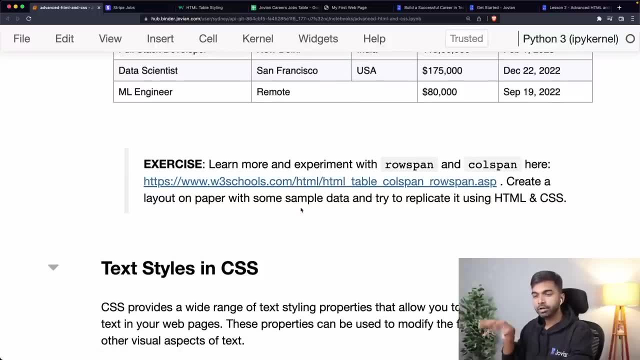 you have to practice, you have to experiment, you have to break things, and only then you understand how things work. Okay, So here's one exercise where you create a layout on paper which contains different Merged cells- Okay, Columns and columns- and then put in some sample data into that layout and try to replicate. 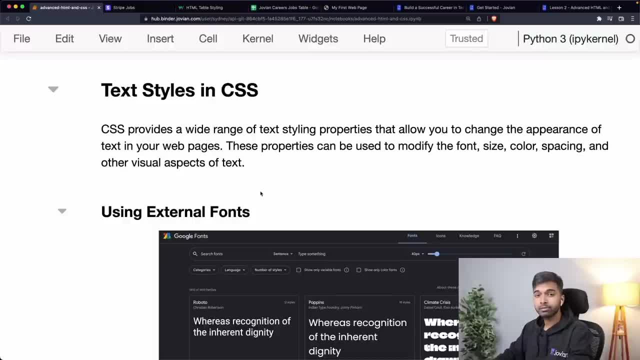 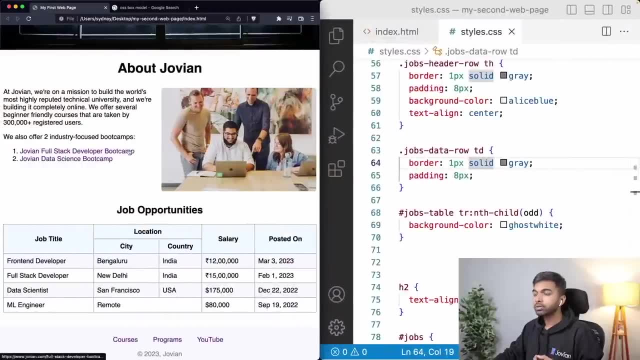 it using HTML and CSS tables. The next thing that we're going to talk about is text styles in CSS, Now that we have set up our table. one thing that we also want to do is we want to improve the aesthetics of this page, And there are two parts to aesthetics. There is 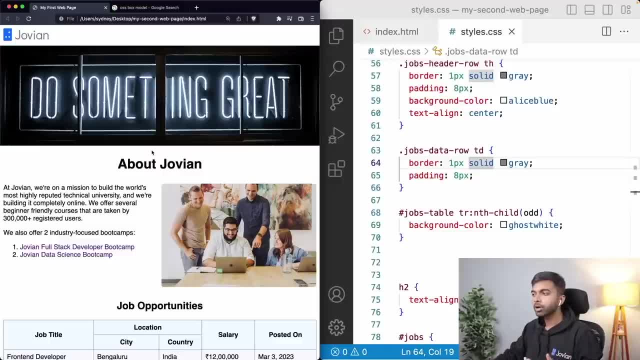 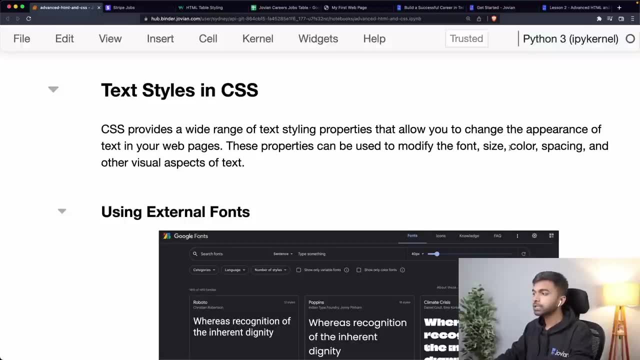 the text, and then there is a colors as well. right, So let's talk about text styles in CSS. Now, CSS provides a wide range of tech styling properties, and they allow you to change the appearance of text in your web pages, And these properties can be used to. 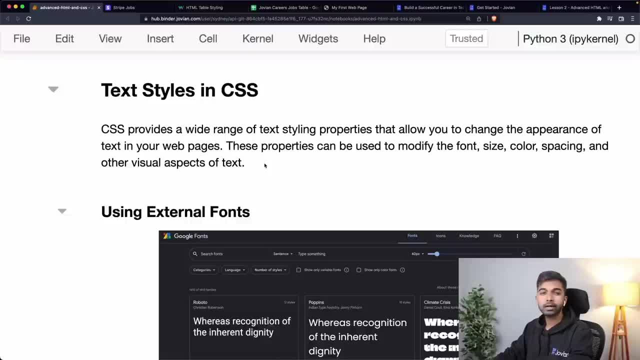 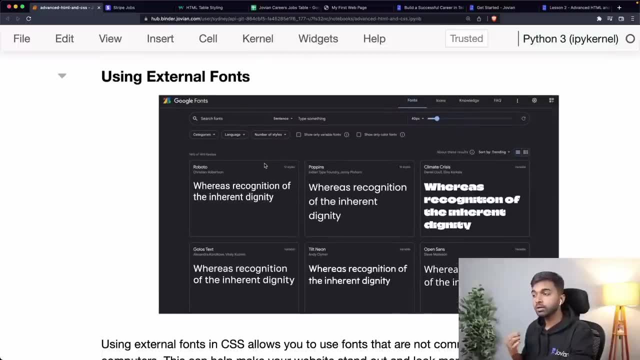 modify the font, the size, the color, spacing and other visual aspects of your text. Specifically, you can use external fonts within your HTML pages using CSS. Okay, Now, why do you want, why might you want, to use external fonts? 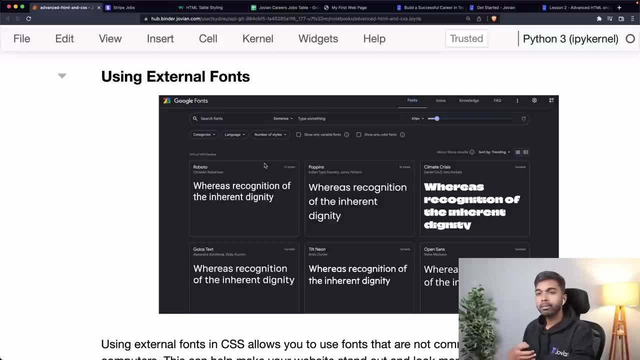 There are some inbuilt fonts that most browsers come with, but that differs from browser to browser And the selection is very small. When you're working for a company, the company may have its own design principles, may have its own design guidelines, may have its own. 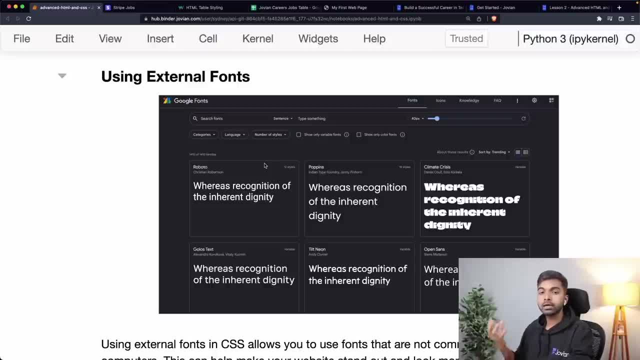 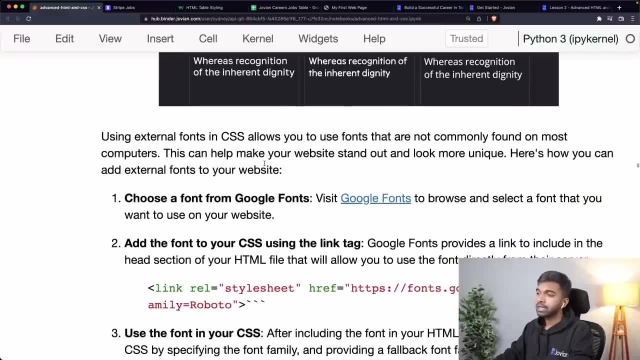 fonts that it is using And you may want to incorporate those fonts into the website, And that is what you use external fonts for. So external fonts make your website stand out and look more unique compared to other websites on the internet, And you can add. 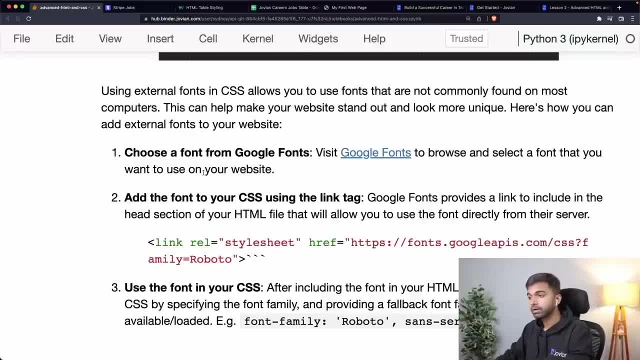 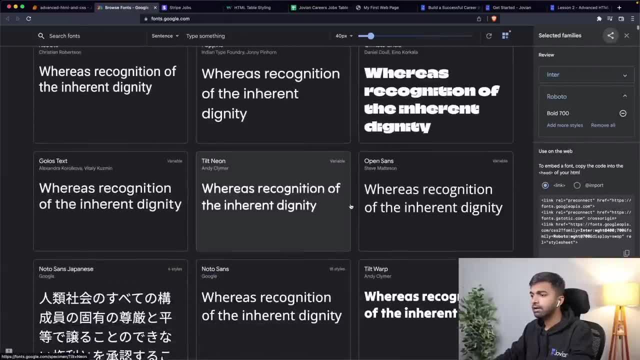 external fonts to your website using the Google fonts web, using the Google fonts tool. Okay So let's visit Google fonts and let's check out some fonts. Okay So, it looks like we have a bunch of fairly interesting fonts here And, of course, there are fonts and all kinds. 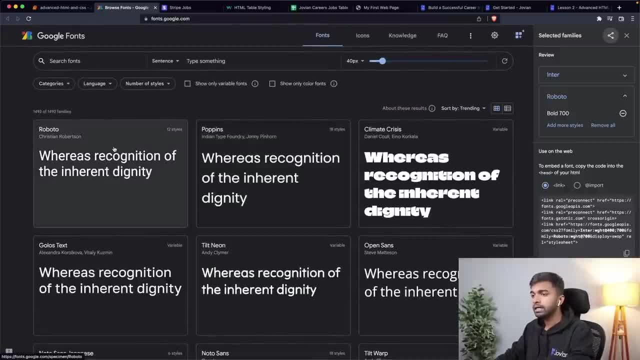 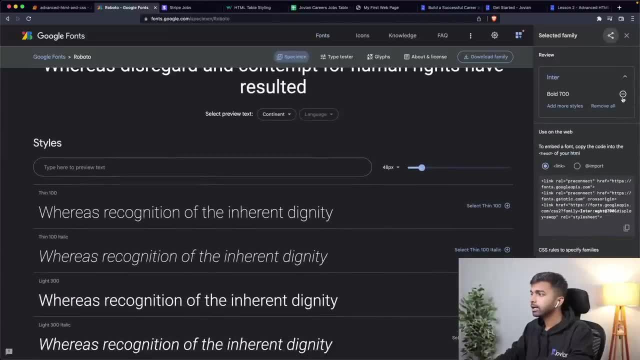 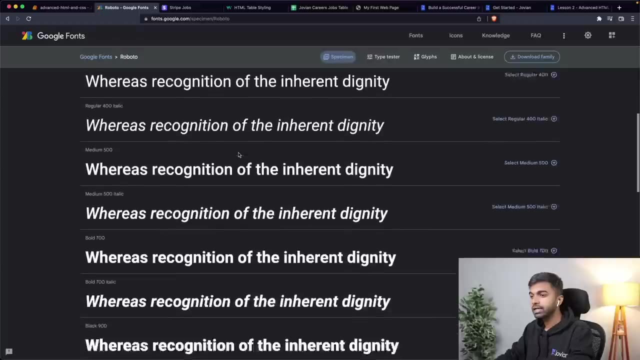 of languages. Now you can click on any one form- For example, I'm clicking on Roboto- and then, once you've clicked on a font, let me just reset the state over here. Once you've clicked on a font, you can then select some styles of a font, So each font can have many. 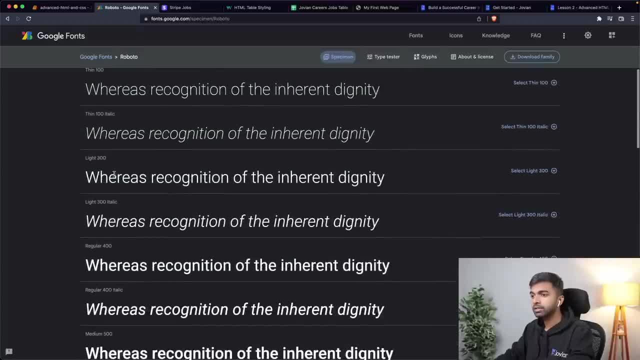 styles. So you can see, here we have the thin font. Okay, So the font is actually a little bit bigger, So let me click on that font. So I'm. we have the thin italic font. we have a bunch of different styles, from thin to thick. Let me just 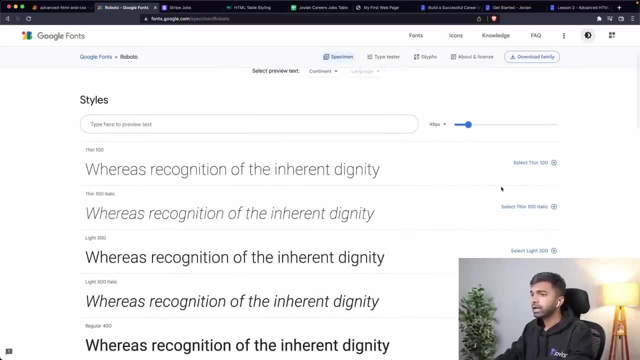 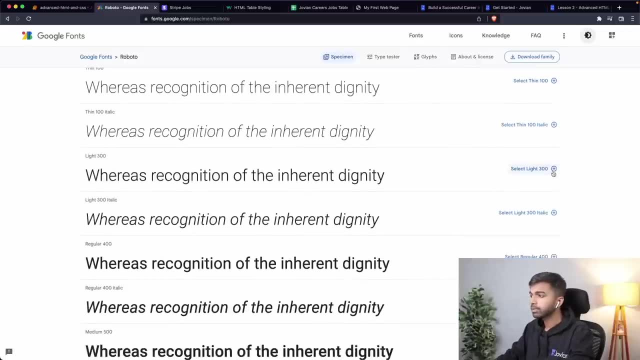 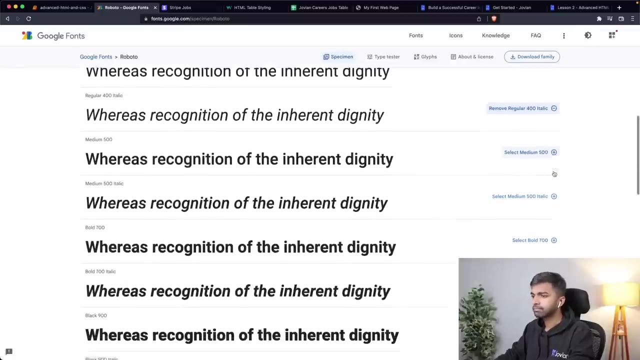 switch to light mode. Yeah, so we have a bunch of styles here And you can then select a bunch of styles. So you can select which styles you want to use in your website. For example, let us use the regular style, Let us use the regular italic style, let us use the old style, Let us use the 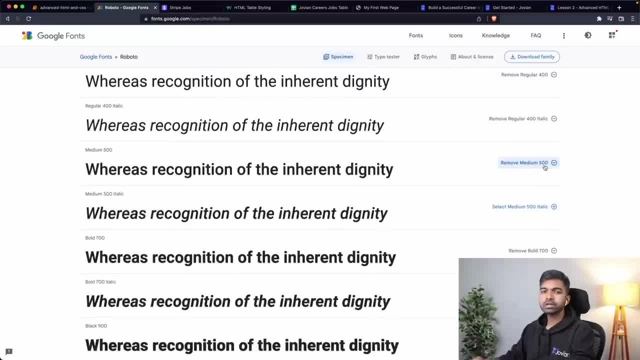 black style And let us use the medium style. Okay, so I've selected a bunch of styles for the Roboto font. this font is something that I want to use on my page, And then there's a button here called view selected families on the top right, And now you can simply copy this code over here. 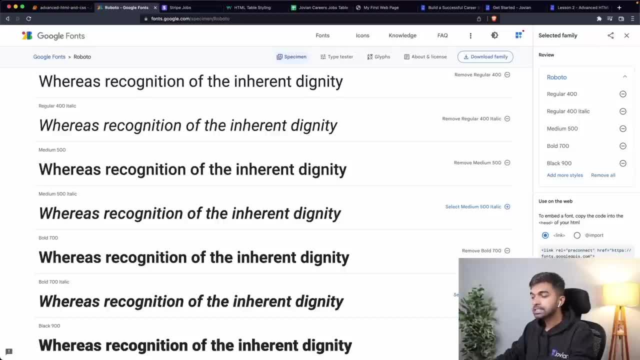 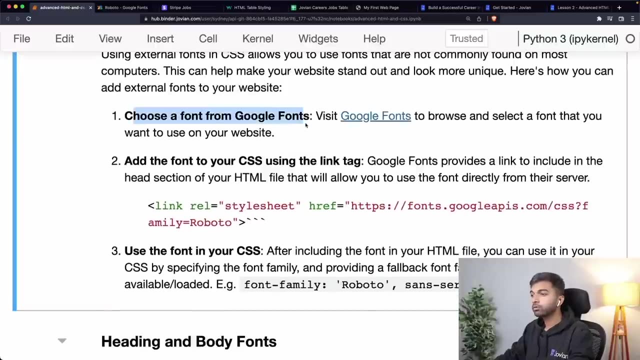 So there's a bunch of code here that you can copy and paste into the head of your HTML page to use these fonts within your site. Okay, so that's what we'll do in just a second, But the basic idea is, if you want to use external fonts, first you choose a font from Google fonts. 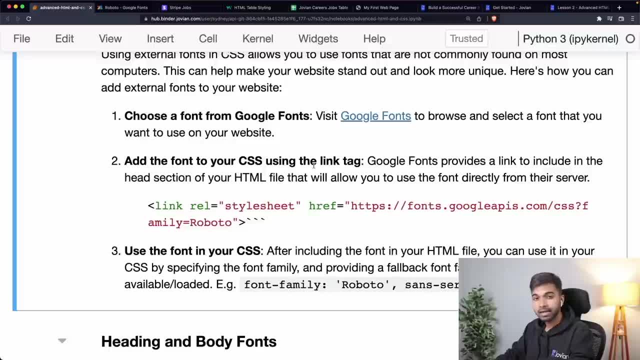 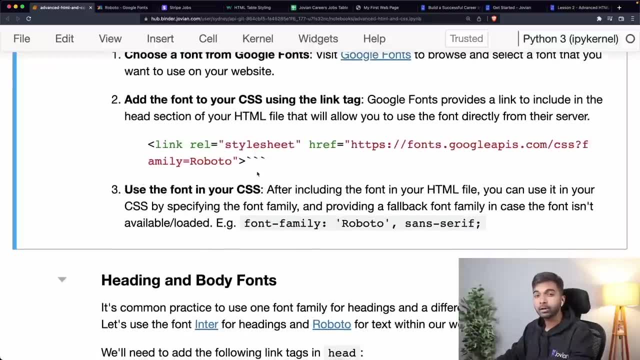 then you add the font to your CSS using the link tag, And we're going to look at that in just a second. Then you use the font within your CSS. So let's say you've incorporated the Roboto font. Now to actually use it on the page for a particular tag, you can select that tag and within 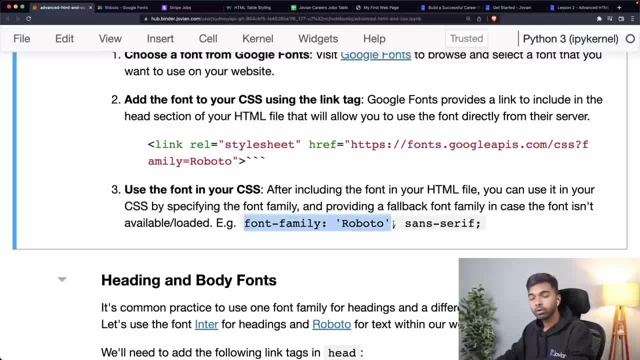 your CSS file. you can simply specify the font family, Roboto or whatever font you have downloaded or included on your site, And that is how you can set fonts for various elements on the page. Okay, so that is how you use external fonts. you find something from Google fonts added. 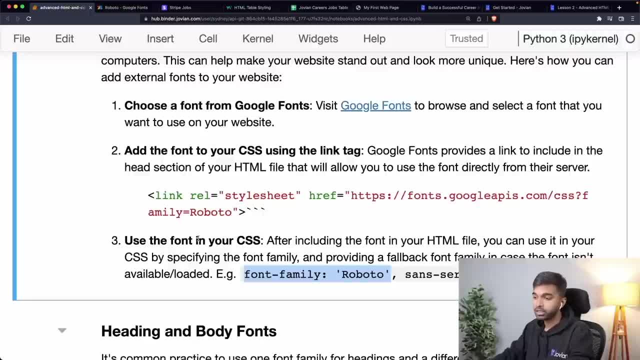 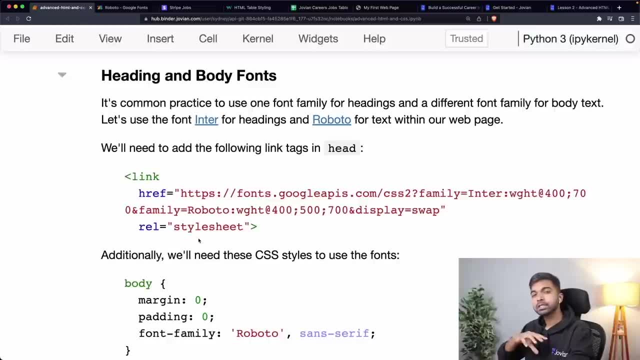 to your page and then just add some CSS properties. Now it is common practice to use one font family for all the head headings and use a different font family for all the body text, And at Jovian we use the inter font. So this is the inter font right here. 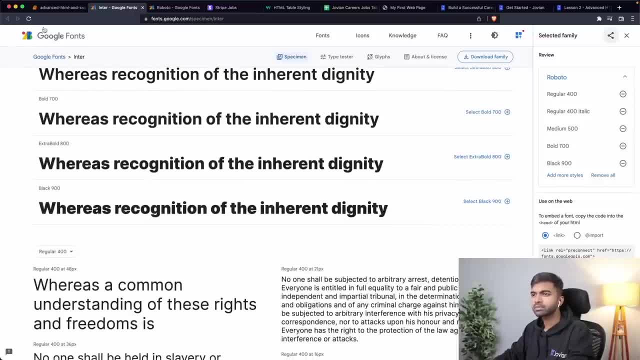 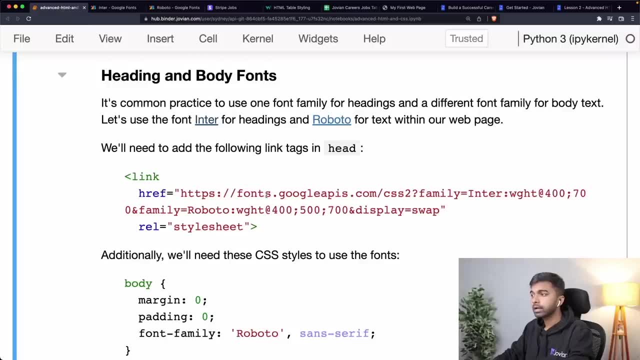 goo, which looks pretty similar to Roboto but has some small differences. So we use the inter font for headings And we use the Roboto font, which we already looked at, for text within our web page. So let's grab a bunch of styles from the inter font. 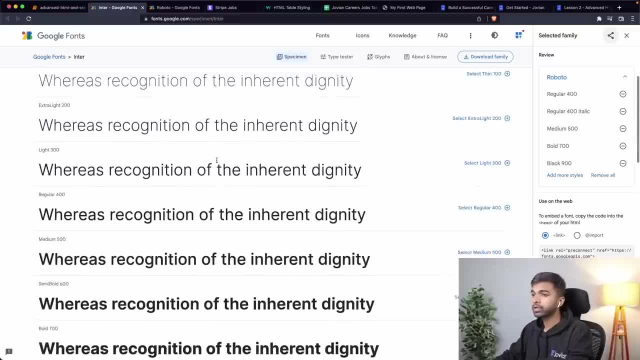 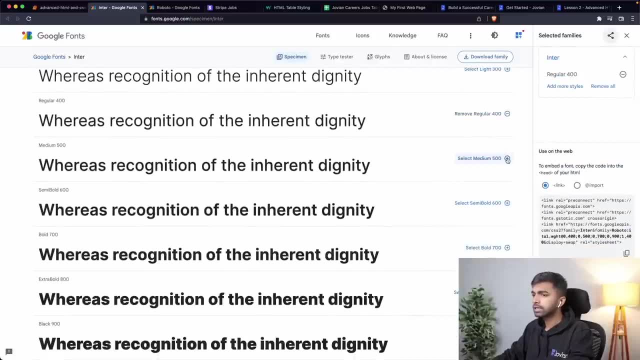 and the Roboto font and then include them on our web page. Okay, But here is the inter font and on the inter font, I'm going to select, let's see. I'm going to select the regular, I'm going to select the medium, I'm going to select semi bold, bold, all of these. 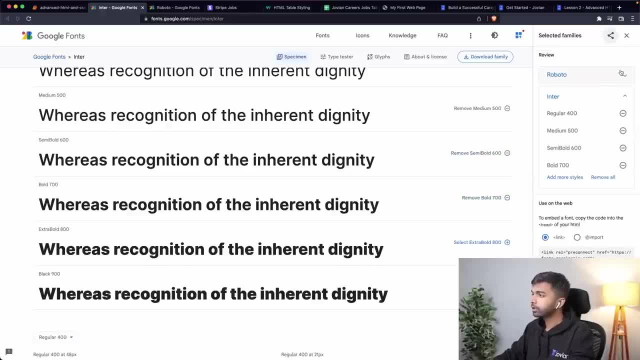 So those are all the styles that I selected from the inter font and from the Roboto font. I have regular medium bold, all right, So now we have styles from Roboto and we have styles from inter, and now I can go in here. 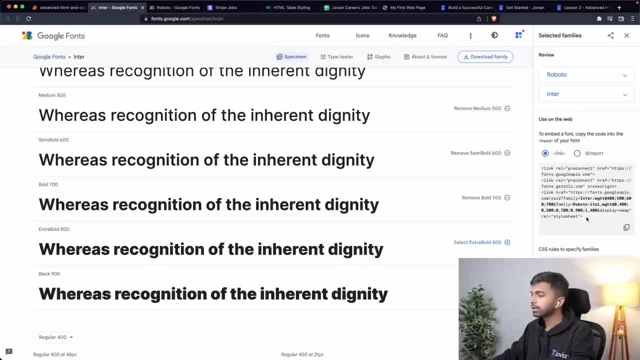 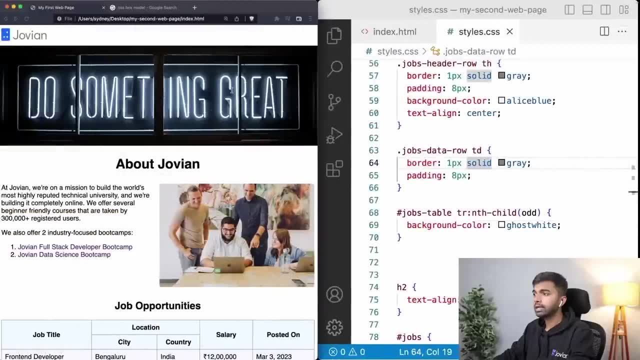 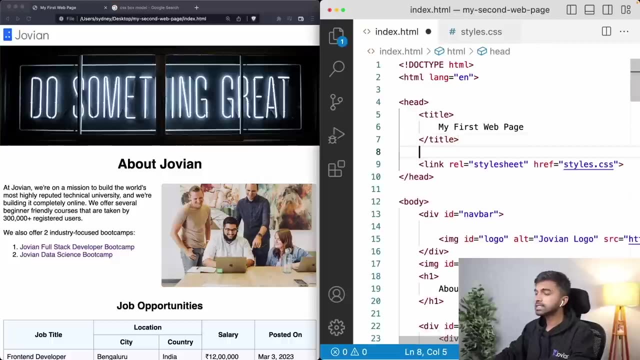 and copy all this. So if you observe this link tag over here, it contains information about which fonts we want to include in our page, And then I can come back into my HTML page. indexhtml come up into the head And before my CSS file I'm going to paste all these link tags. 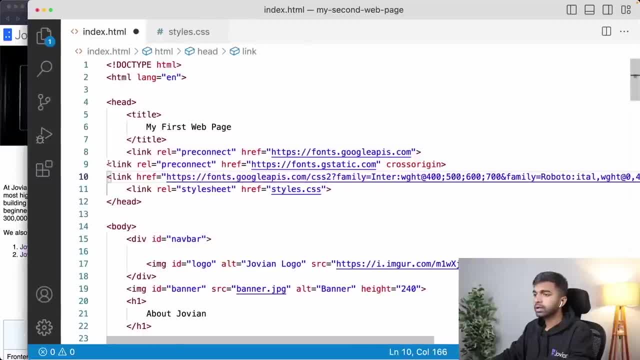 Okay, So just to show you what that looks like, it looks like we have added a link tag called pre-connect and two of these pre-connect tags. One goes to Google APIs, one goes to G static, not something we need to worry about. 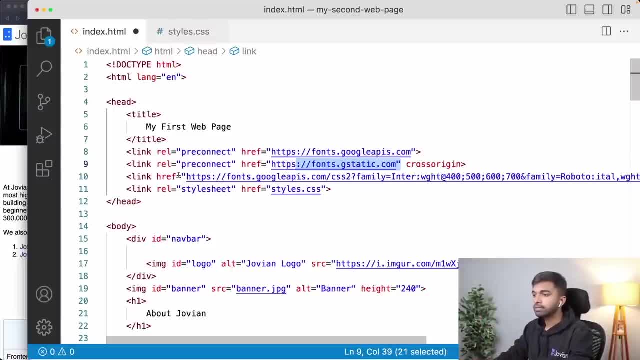 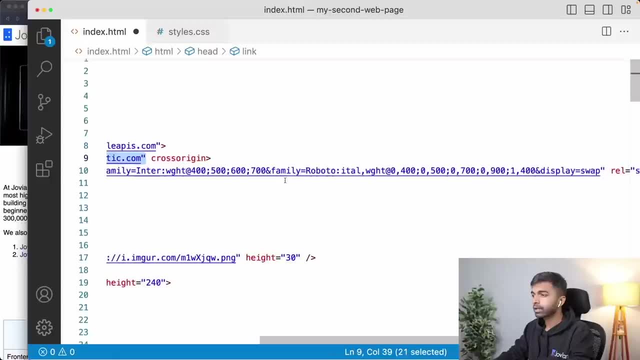 We just have to paste it in. But here is the interesting thing: We have this link tag which contains the link to Google fonts, and it contains these font families: inter and Roboto. We have these font families and these font families are included as a style sheet. 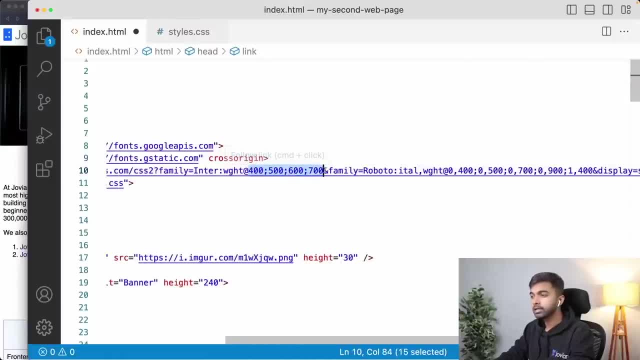 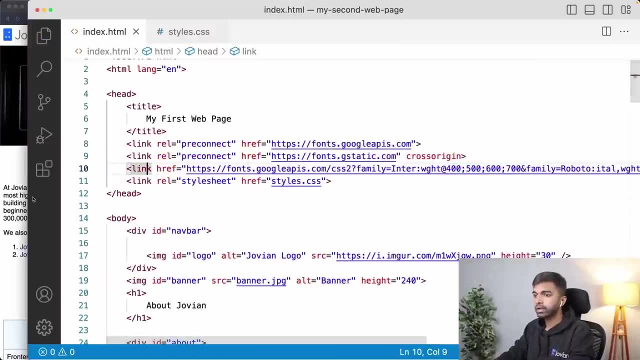 Okay, And in in each of these font families, various weights are also included, So you can actually go in and edit this URL slightly in case you want to include different weights. but I'm just going to save this now And at this point the fonts have been included on our page. 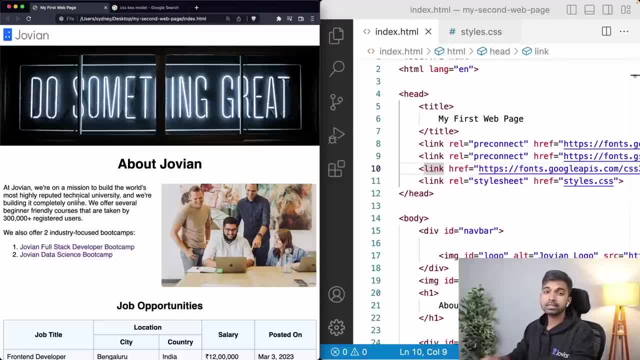 Okay. So if I reload the page, you can see that nothing has happened yet, because I've simply included the font right now. The next thing I need to do is actually use this font on the page, And that is something that we're going to do in the CSS file. 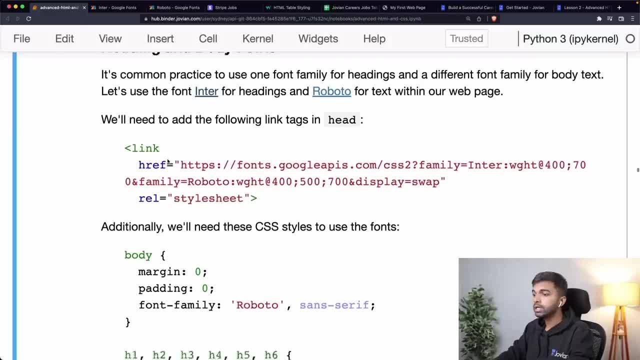 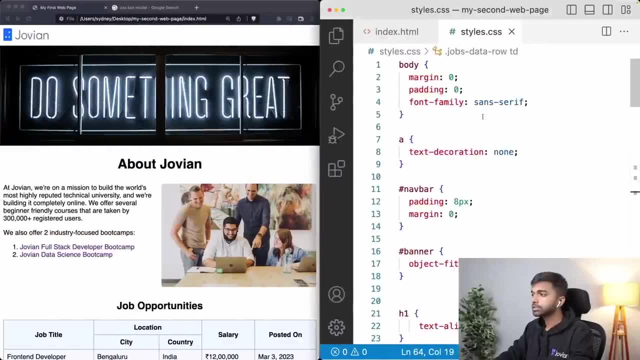 Okay, How do we do it? Well, we need to add the font family for the body, And then we also need to add the font family for the headers. Let's do that. first I'm going to add the font family for the body. 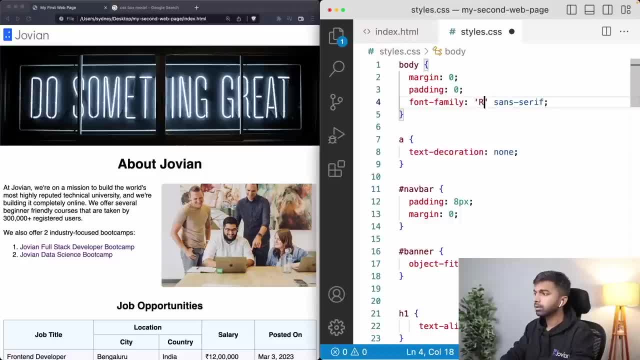 So let me change this to font family- Roboto. Okay. So what we often do is we specify a font family for the body, but in case this font was not loaded properly, in case the request failed or something, we also specify a backup as. 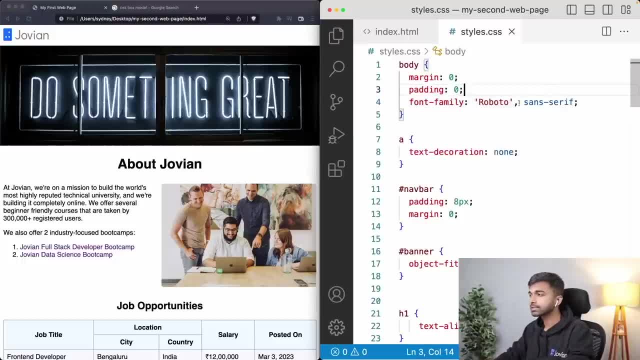 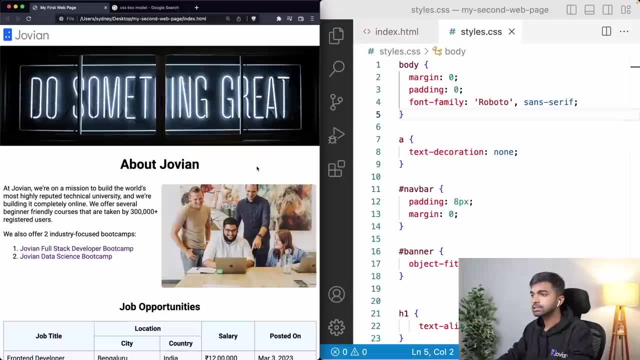 one of the default font families from that are already present in CSS, So in this case the backup is sans serif. Okay, Then I am going to just reload the page after saving this, Okay, And you can see that there was a small change in the font. 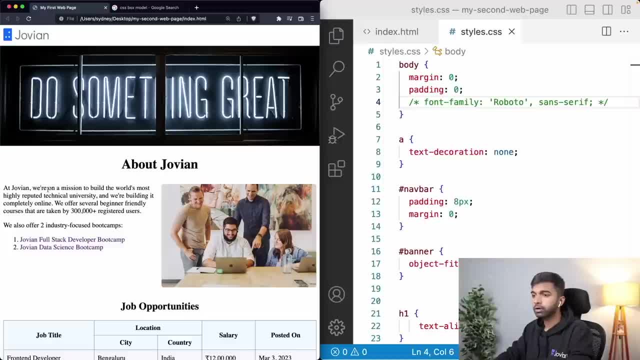 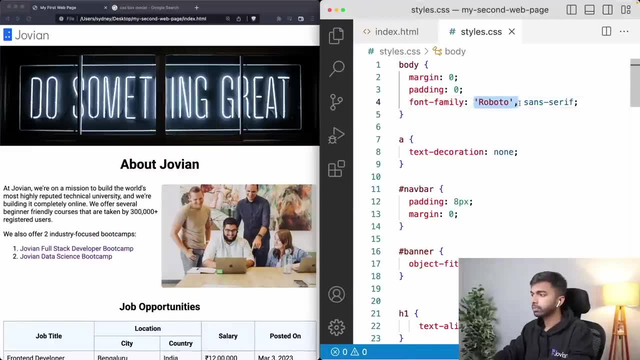 So if I disable this and reload, you can see that the font looks different. And if I enable this and reload, you can see that the font looks different. And if I remove Roboto, you can see that font looks slightly different. It's a very slight difference. 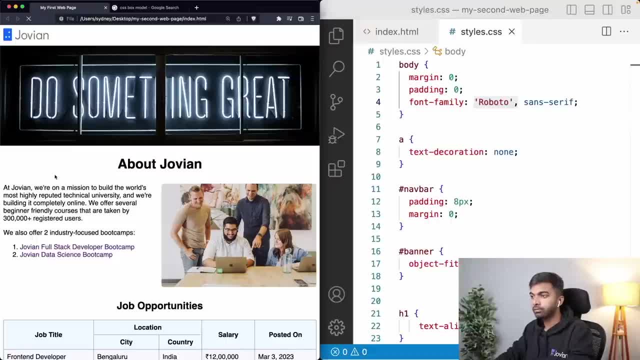 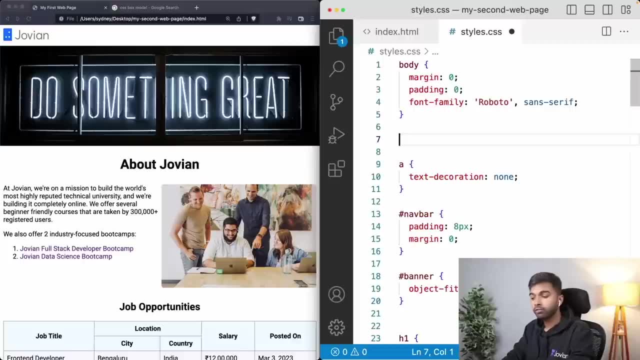 All of these fonts are very similar often, but Roboto is what our design team has told us to use, So that's what we are going to use for our body- Great. Next, let us set a different font. Enter for the headers. 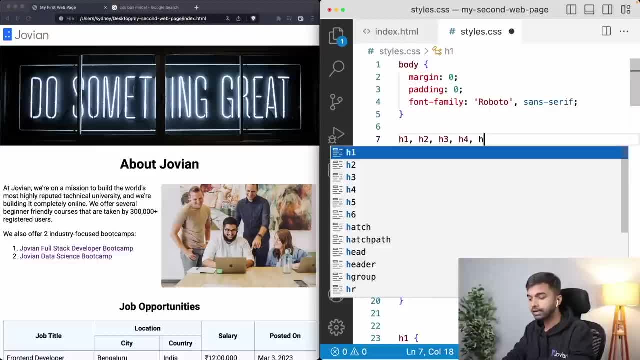 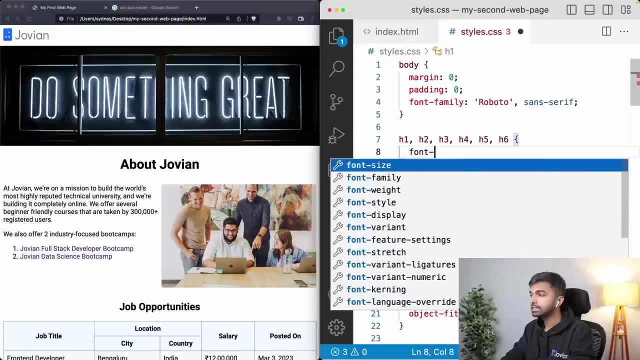 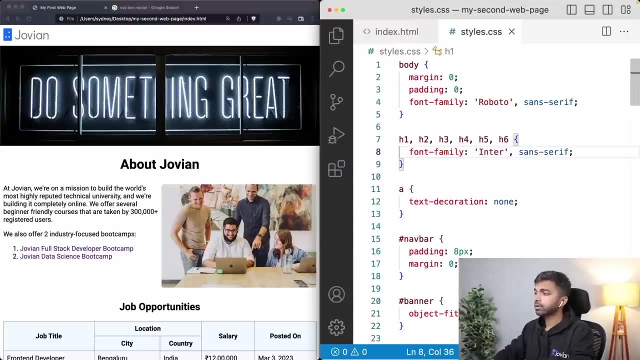 So let's select H1, H2, H3.. So you can also select multiple tags like this using commas: So H1 to H6, we're going to apply this style to all of them And let us set font family, enter and let us set the backup as sans serif. 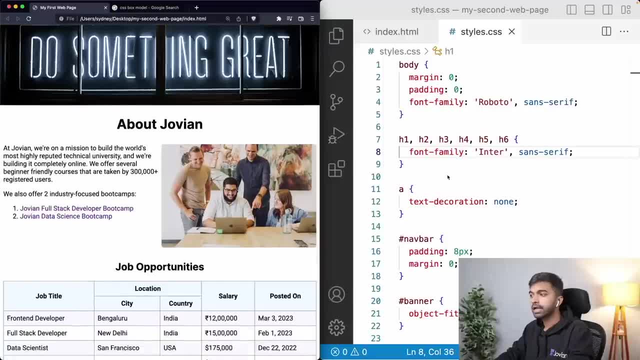 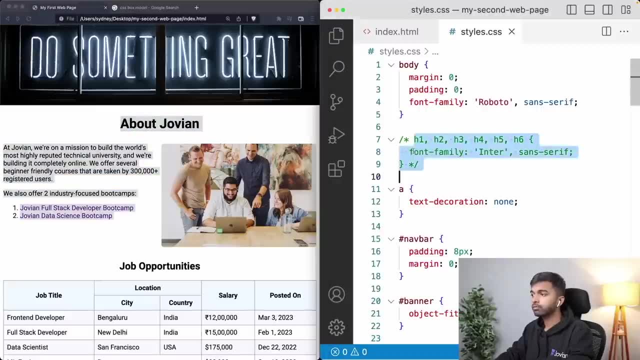 Okay, And let's reload. And now you can see that again there was a slight change, If I show you. So this is without the inter font family And this is with the inter font family. Okay, Slight changes, but it looks on brand. 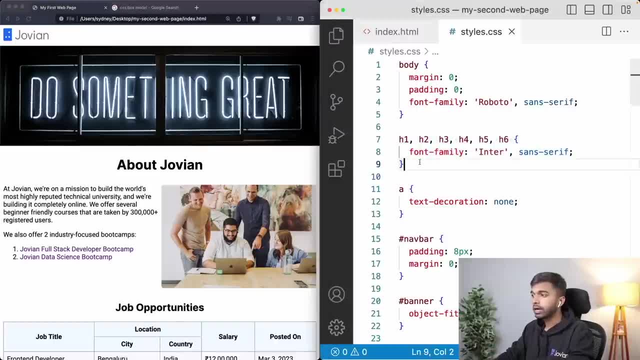 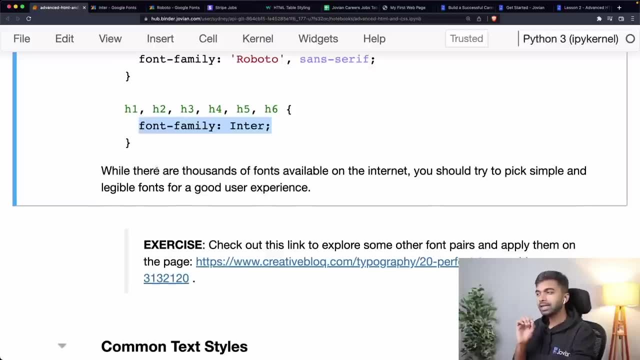 It looks closer to what we have elsewhere on Jogin. All right, So that is how you use external fonts. Now there are thousands of fonts available on the internet and you should try to pick simple, legible fonts for a good user experience. 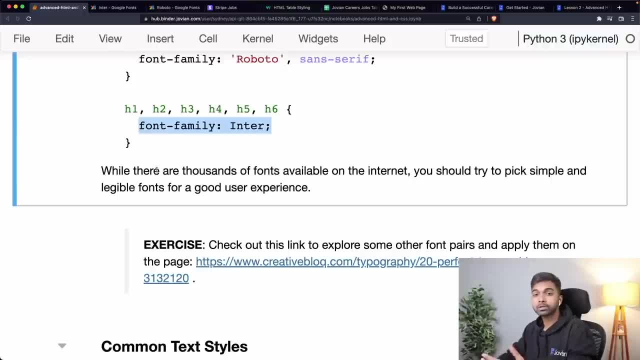 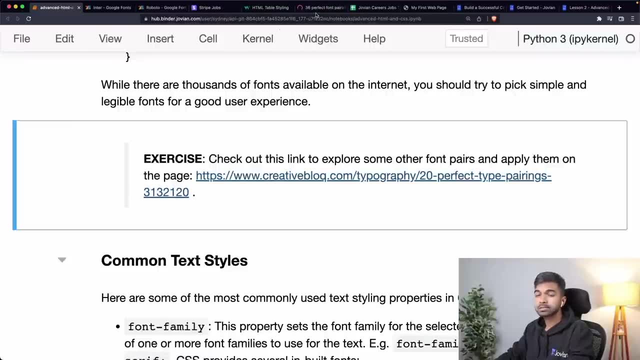 Otherwise you might run into issues where people are not able to actually read what's on your site, even though it looks pretty. So check out this link to explore some other fonts. Pairings- So a header and a body font pairing is often called- is often. 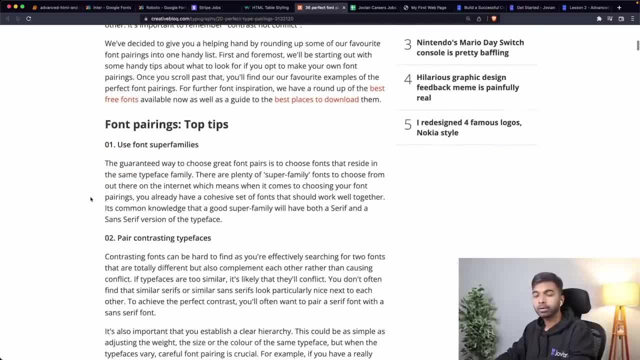 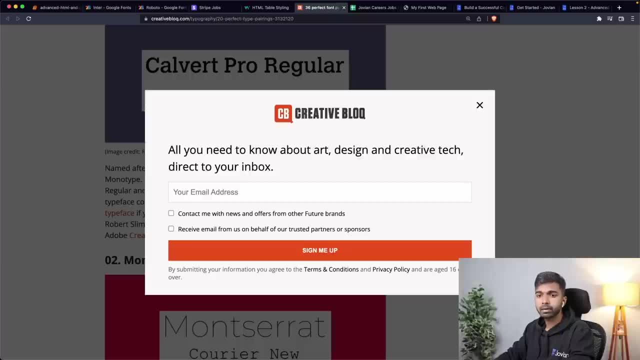 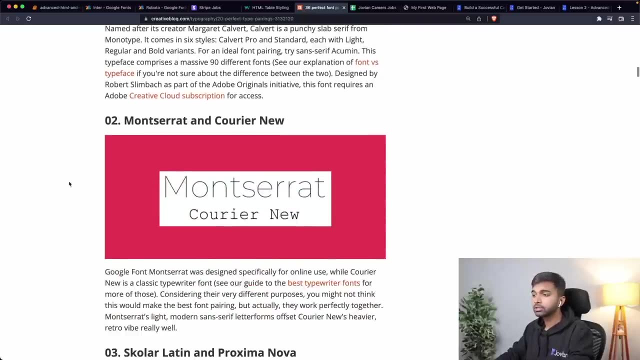 So there are many header and body font pairings that people have created by looking at Google fonts, for example, Calvert and acumen, So this is a good combination. Yeah, Calvert, Calvert and acumen is a good font combination. 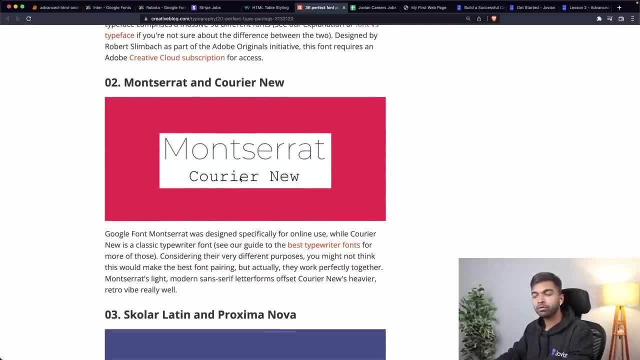 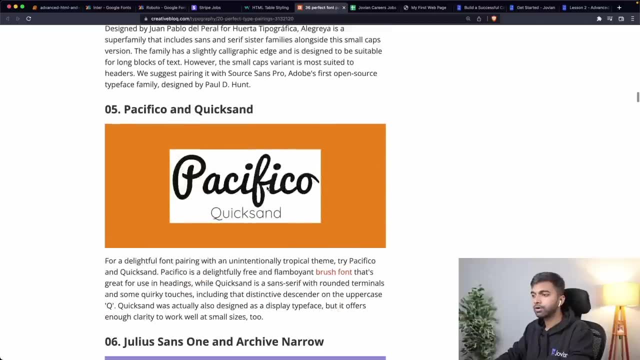 Monster, art and courier is a good font combination, but obviously it looks very different from what we have. Then we have a bunch of these. These are serif fonts, These are not science serif- and we have these more interesting fonts. We have some fairly nice cursive looking fonts. but depending on what you want, you can use. 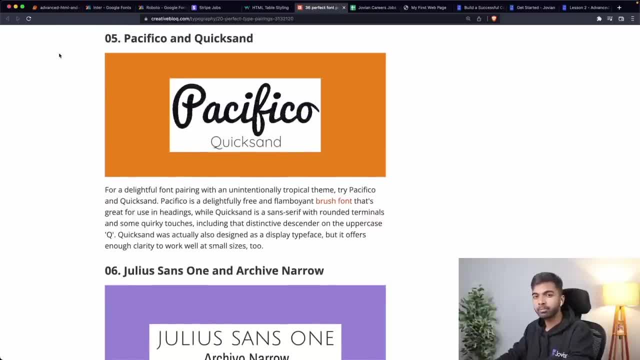 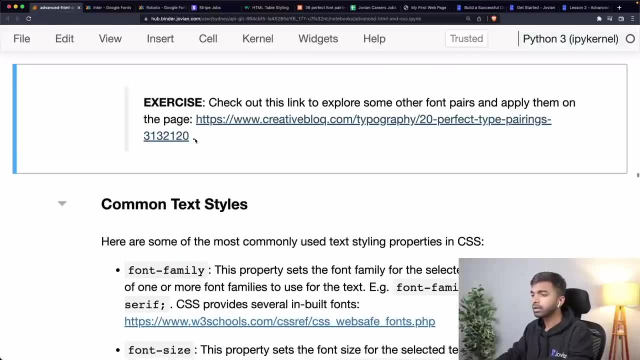 various fonts on your webpage, and I encourage you to experiment, but also be conservative. stick to some of the more standard types so that people can actually understand what's on your page. Now, apart from the font, of course, there are many other textiles that CSS also offers. 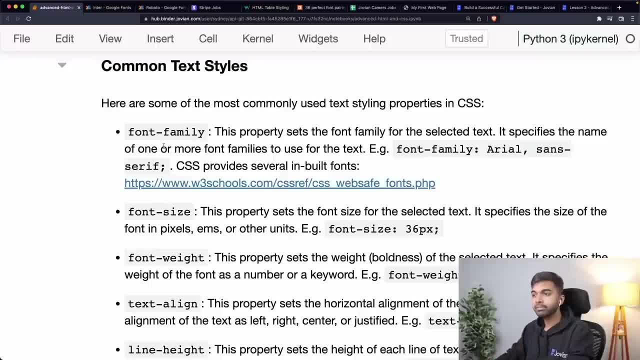 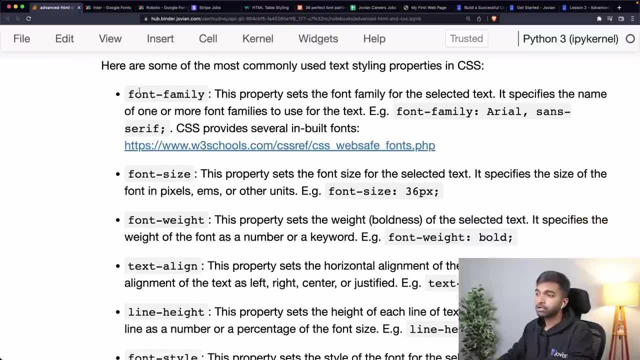 and we're just going to run through them very quickly. We're not going to cover everything necessarily, but I encourage you to explore these and experiment with these as you are working through the lesson. So the first is font family. This is something that we've already looked at. 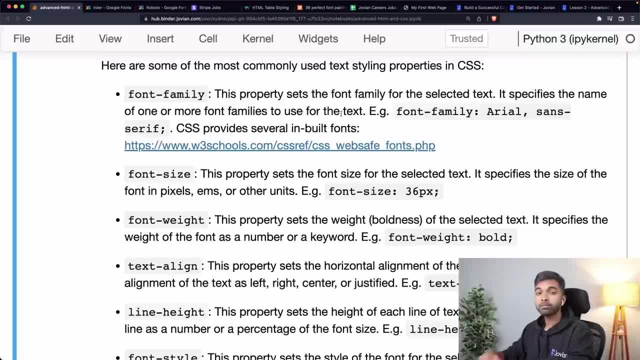 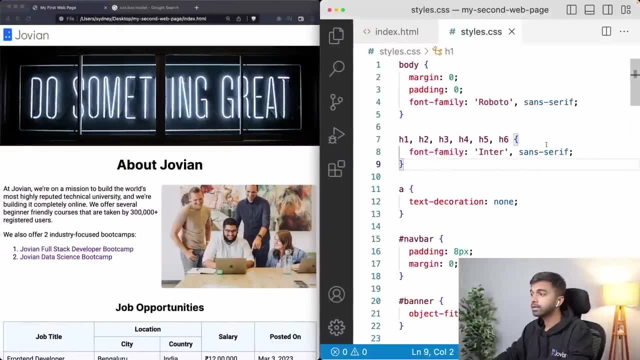 It select, it sets the font family of the selected text. We set a font family for the body and then we over wrote that font family. So we set a font family for the headers as well, And the specific setting for headers will override the setting from the body, which 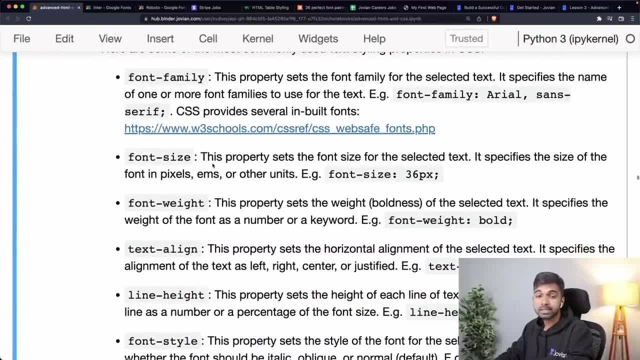 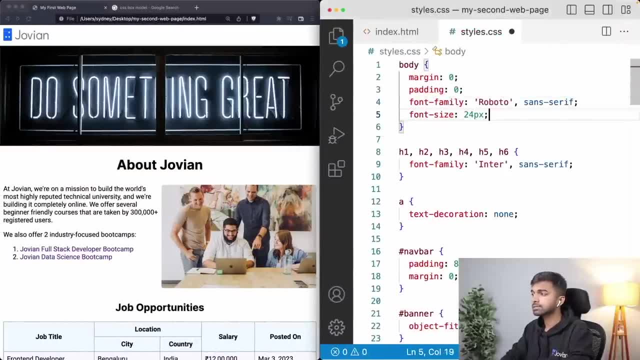 is applied by default. Yeah, So we have a font size so we can actually go in into the body and we can change the default font size. So let's say I set the font size to 24 pixels and reload the page, You can see that all the fonts have become slightly bigger. 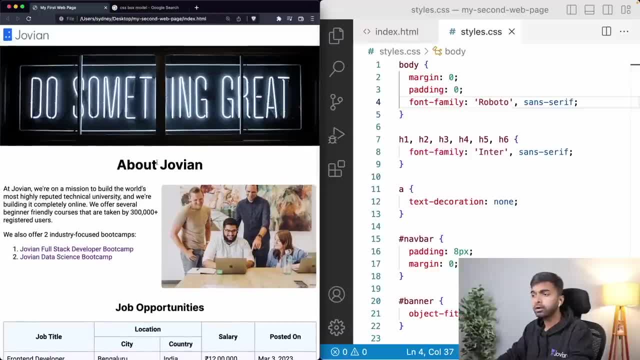 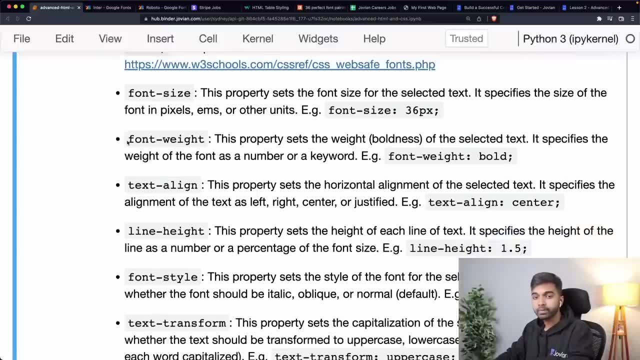 I'm going to keep it to what it was earlier, the default. Now there are many ways to specify sizes and we look at those as well. Then we have the font weight, So we have a bunch of properties that we can use to set the weight or the thickness of. 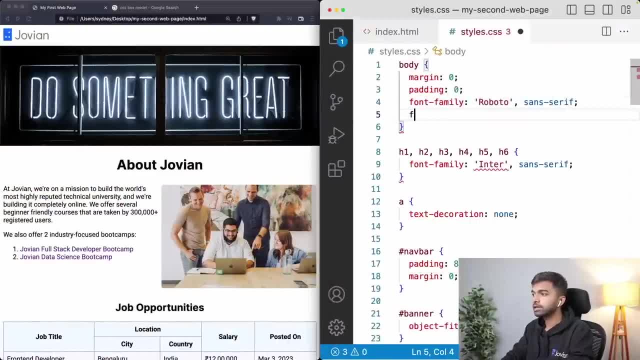 the font. Okay, In terms of the body. So if I, if I said font to weight to 400, that's basically the regular font weight, but I can set it to 600 and then it'll be slightly thicker. And I think we included a bunch of other font weights as well. 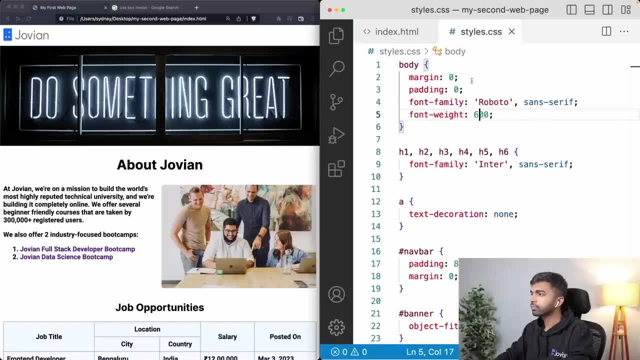 Let's see We also included 500, 700 and 900.. So let me select 700.. Okay, That's about the same. Then let's select 900.. That's really thick. We also have 500, which is like a medium weight. 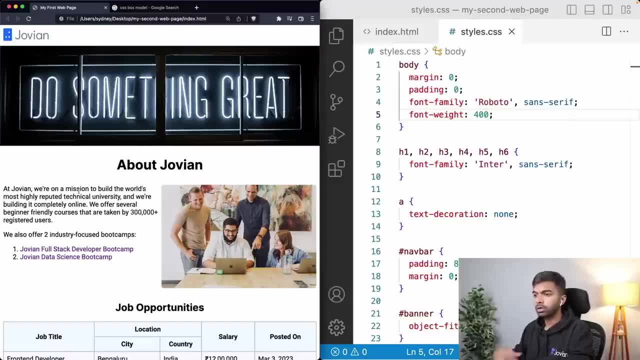 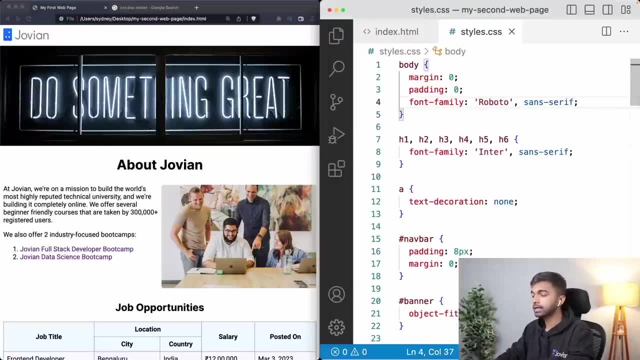 So that's a less, less thick, depending on what you want to convey, how prominent you want the text to be. You can set a font weight, and 400 is the default, but you can set a bunch of other font weights as well. 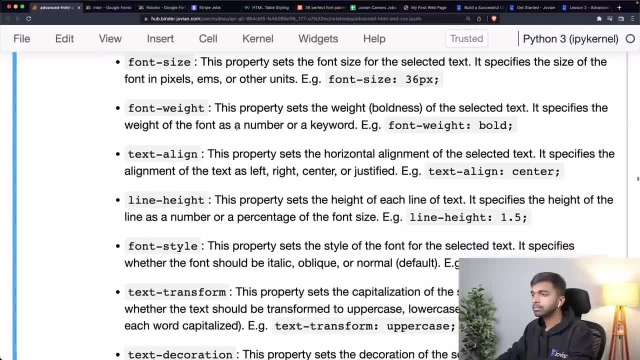 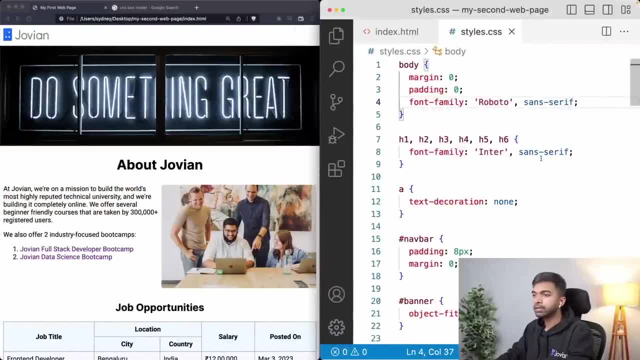 Okay, And we look at a few examples of font weight. Then we have the text align property, So the text line, of course, is used to do a center alignment, left alignment, right alignment. So you could say, for example, text: 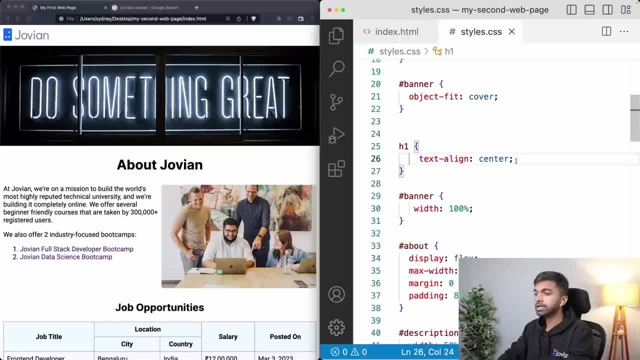 We've already done this here. We've done H1, text line center. We could have changed this to text line right And then the text would be right aligned. We could set it to center again and that would be centered again. 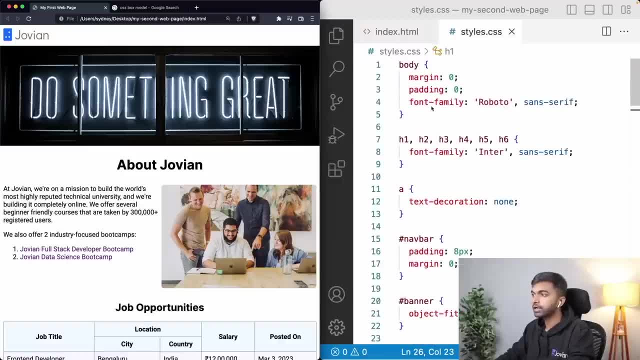 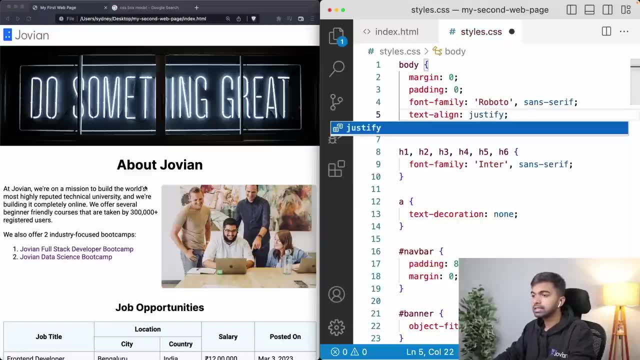 So alignment is just left, right center. There is also an alignment called justify, which is often used in text. So we say: text align, justify. What that does is: you see this empty space at the end of the line? It makes sure that all lines there are no empty spaces at the end of the line. 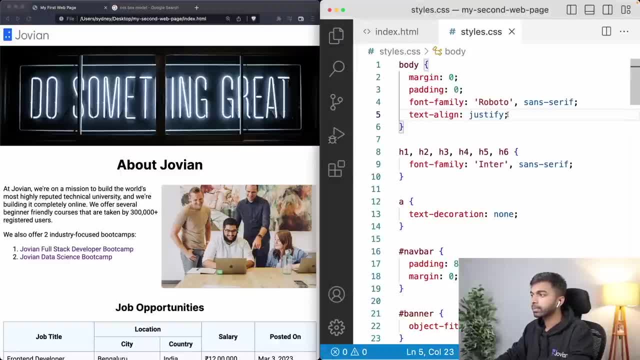 And all the spaces distributed between the words. So you can see now. I said text line justify for the body and all the spaces now added between the words. This is not very readable So it's generally avoided unless you have to ensure that there is no space at the end. 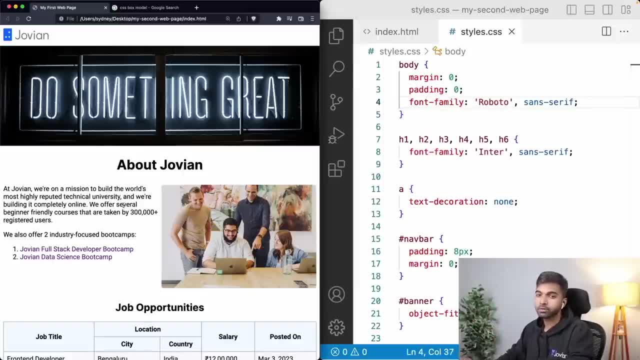 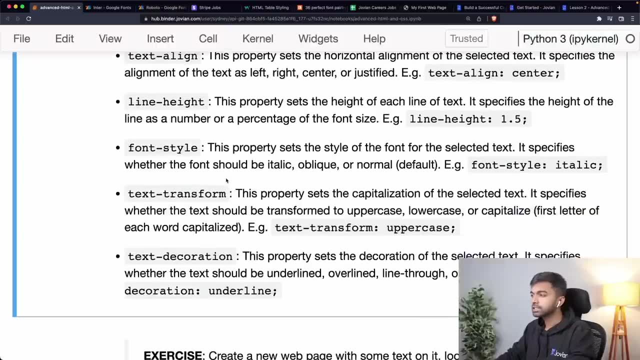 of the text. So I wouldn't do it, but it's a it's an option for you. So you have left, align, center, align, right, align, justify all of that. Okay. Then you have the font style. So the font style is used to maybe make things. 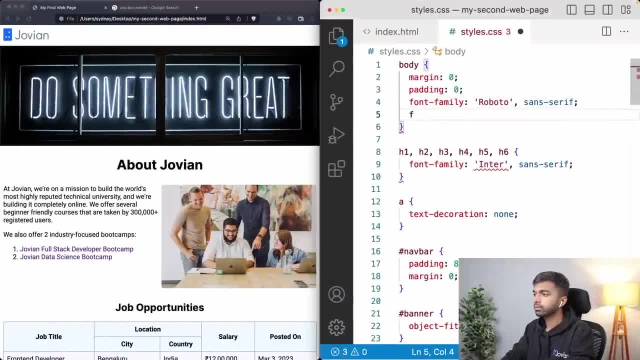 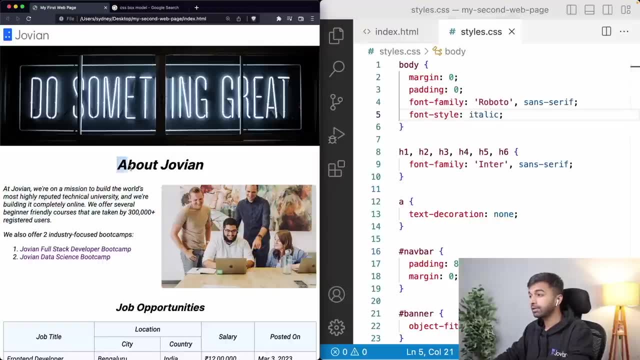 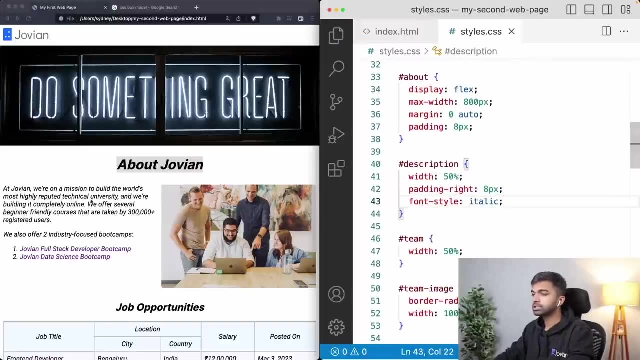 Italic, So I can say font italic and you can now see that everything is a little italic, everything on the page. You can of course also apply it to just a specific section, So I could just go into the description here and I could just apply the font style italic. 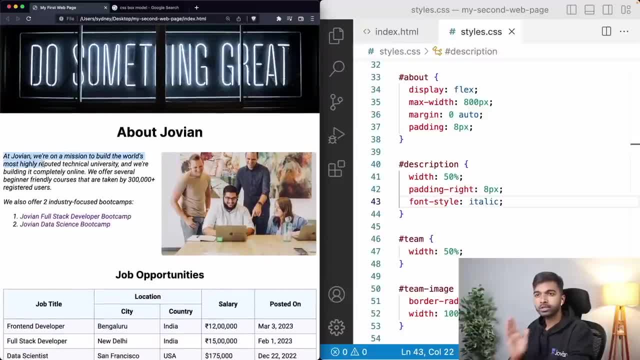 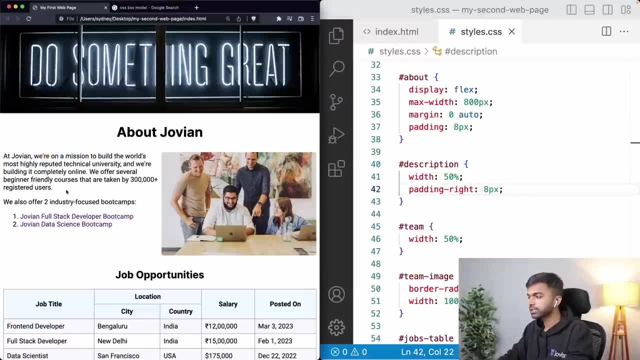 so that everything else on the page is normal. but this is italic, which is just slanted to the side, And there are a bunch of other font styles as well that you can apply. Okay, Well, encourage you to check it out. 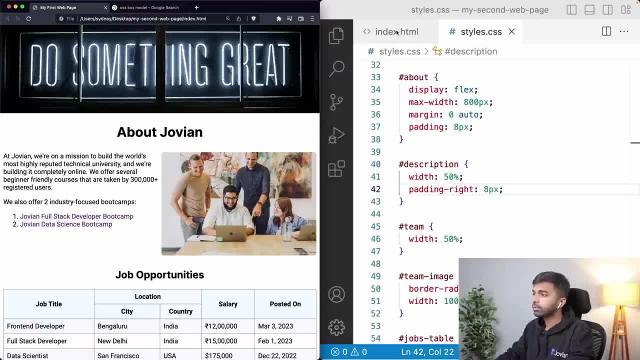 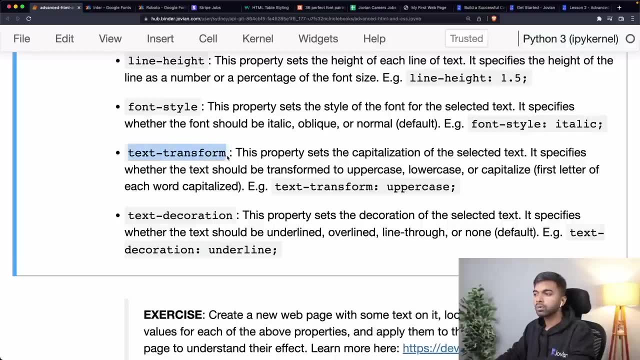 There are a bunch of different font styles. You can use What else? Well, we have a text transform. so text transform can be used to automatically make the kill, Make all the texts upper case, For example. let's say we wanted all our headings to be all caps. 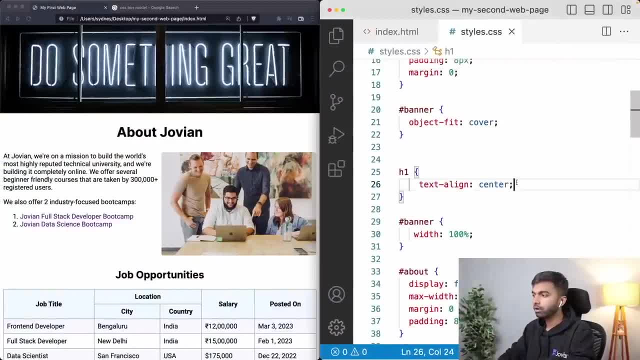 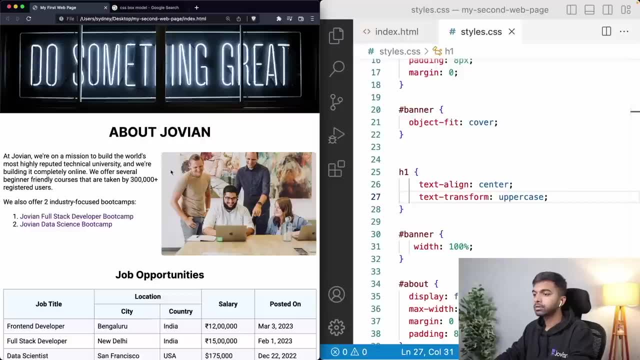 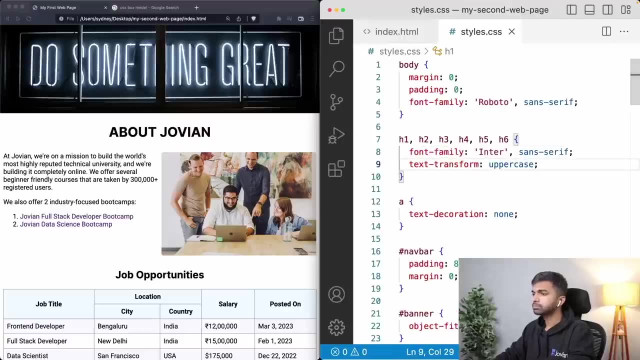 So we could, of course, type it in caps and HTML, or we could just set text transform upper case, And now all our headings would automatically be uppercase. Of course, this is just for H1, but I could go in here and apply it to all the headings. 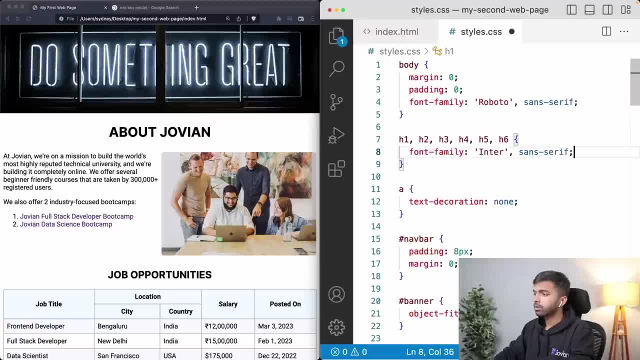 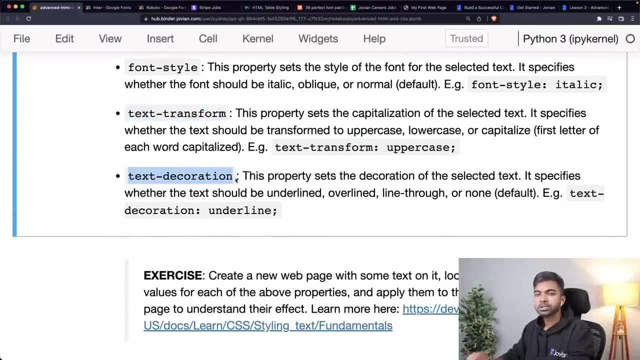 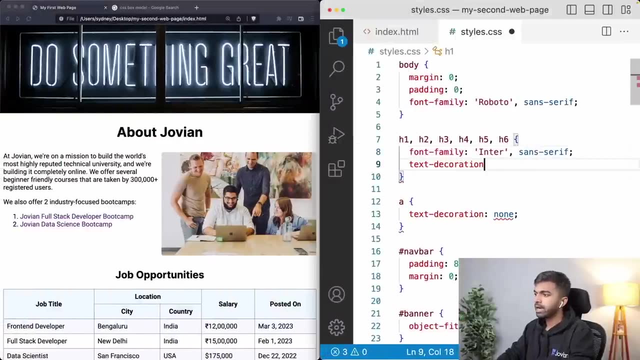 and now everything is uppercase, All right. So that is text transform And finally we have this text decoration. So text decoration is used to add a line, whether you can have a underline, overline or strikethrough. So I could go into the headings and let's say I want my headings to be underlined. 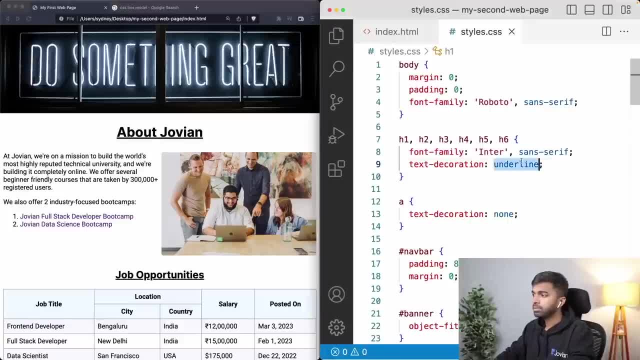 So now the headings are underlined, or maybe I want a line over my headings. Not sure why I might want that, but it's possible sometimes for certain designs that might be useful and you could also have a line through it. This can be useful if you have specific things within the text that you want to strike out. 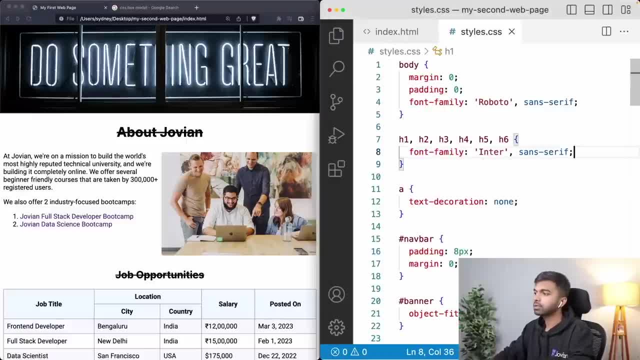 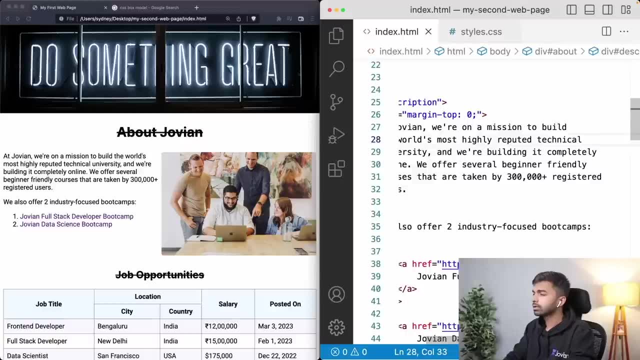 So you could put a span around some text and then just put text decoration line through. Let me show you a quick example. Let's come in here into the description and let's say we want to change this to. we want to strike out most highly. 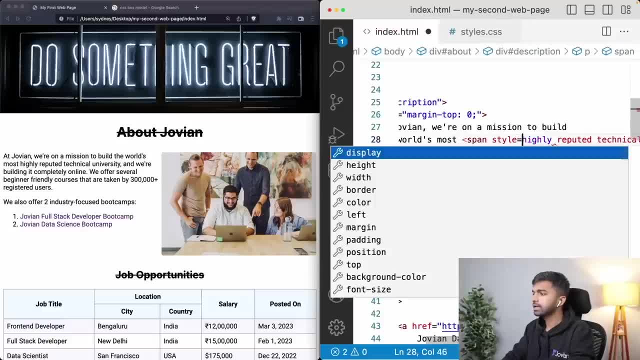 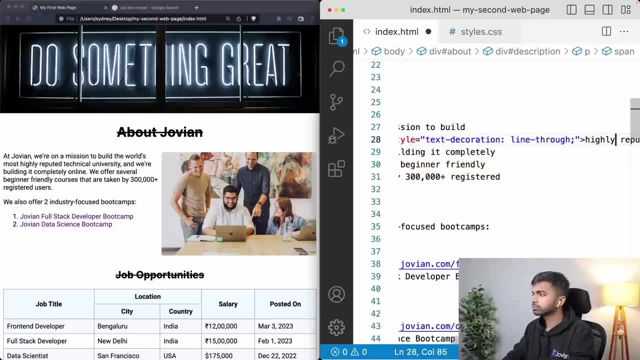 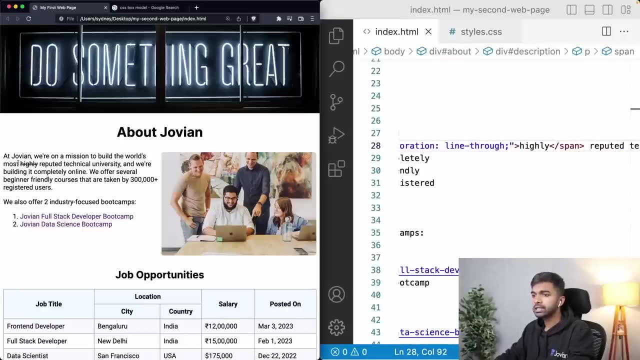 So I could just put a span here and I could say: style equals text, decoration, line through, and I could close the span. All right, So now we've put this span and now you can see that the word highly is struck out, as we might expect. 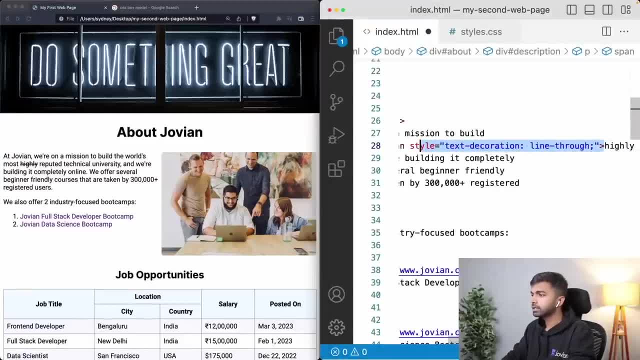 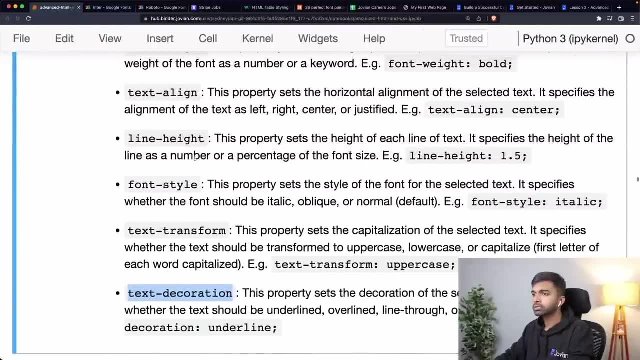 So that's how you can use this text decoration line through. Okay, So that's just one of, or these are just some of, the properties. There are many, many more. One other that you might use from time to time is the line height. 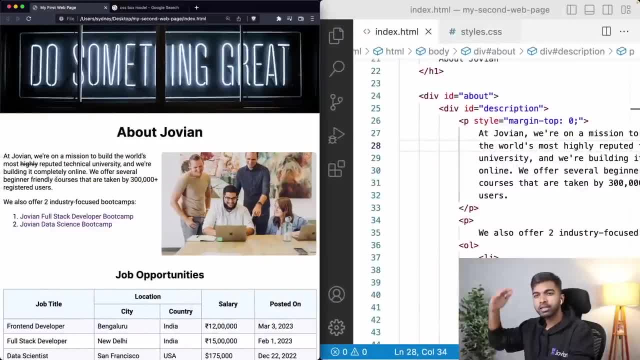 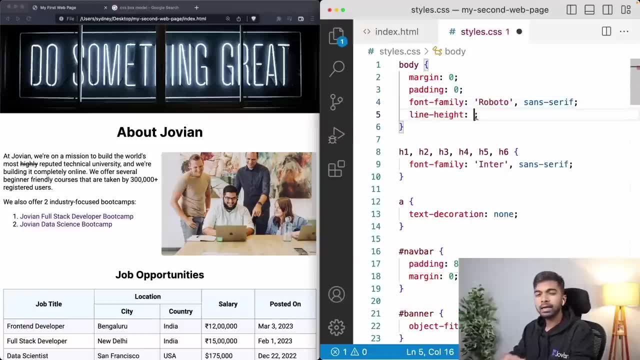 So you can see this text over here. If we want to make sure that maybe there is more space between the lines, we could set a line height. So we could come in here and we could set a line height. And the line height is normally expressed as a single number, which is a fraction of: 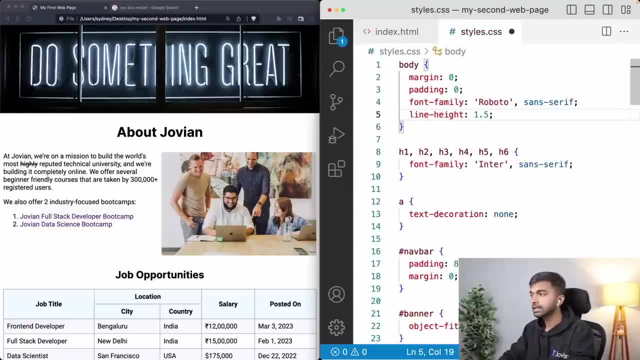 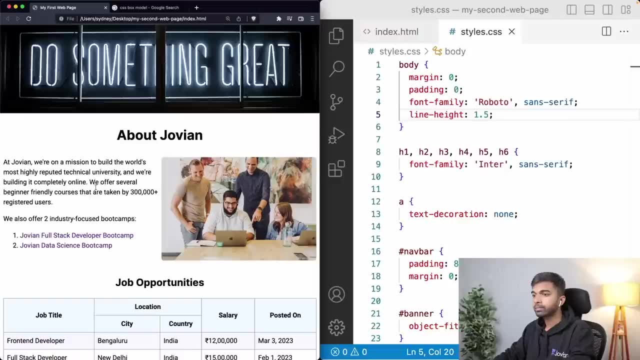 the point size. So let's say we want the fraction of the font size. So let's say we want a line height, There'll be 1.5 times the normal font size. So if I just do that, you can see that now everything is a little more spaced out. 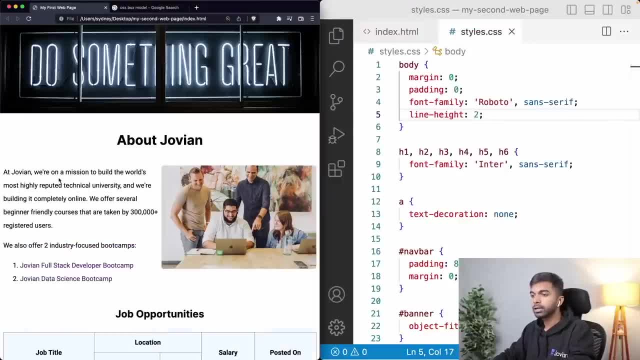 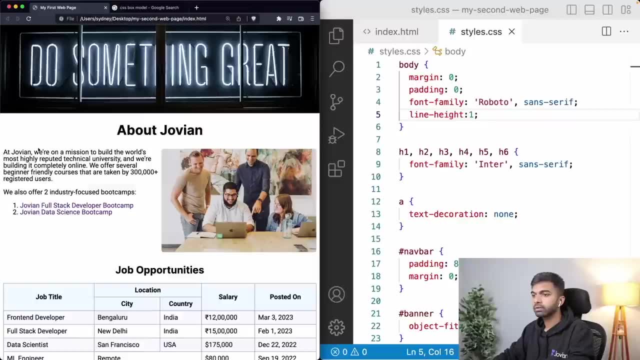 If I set it to two, so then there's going to be almost a double distance between each line, or I can just set it to one, and then everything is going to be very close together. That's probably not what we want. Something around 1.2 is the actual line height that is set by default. 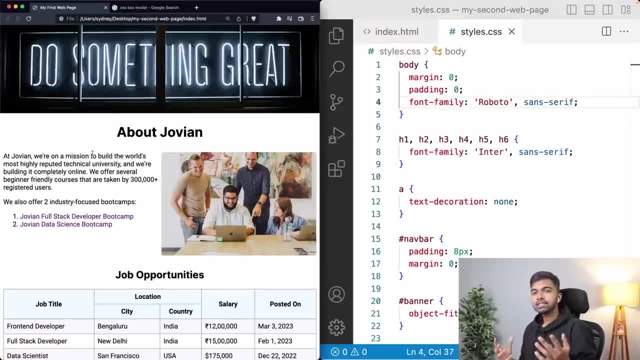 So that's what you might want to stick with. Okay Again. So these things are properties that will be defined in the design system or in the design mock-up that will be shared with you by a designer at your company. But it's good to know what each of these do and you can experiment just to visually see. 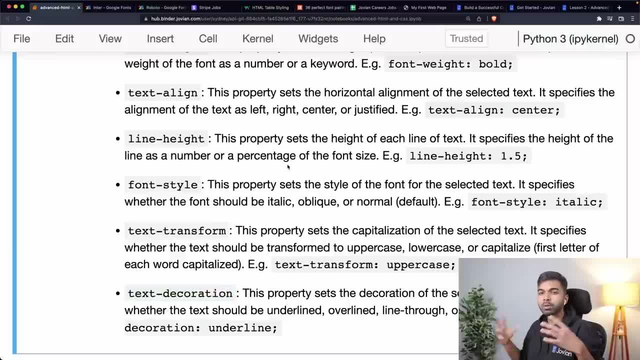 what looks good. You might have the question: given so many properties, so many values, how do I decide what to pick? Well, keep it simple. just use as few properties as possible and then introduce properties one by one. If they make things better, you don't have to add all these properties necessarily. 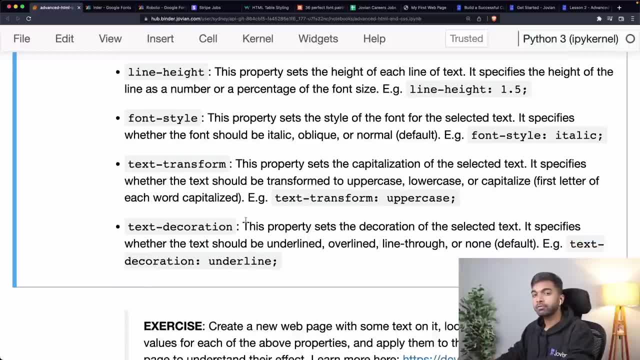 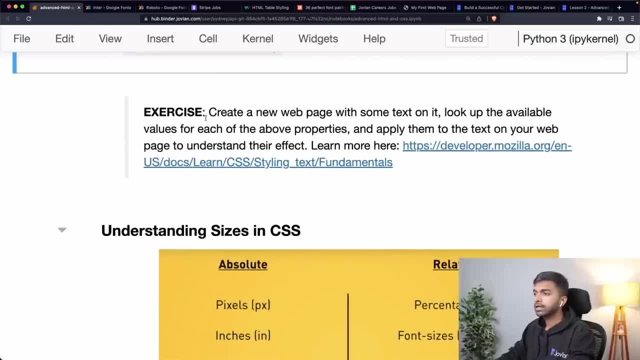 And, of course, most of the time, you're going to be using some kind of a framework which will have all of these properties configured by default. Okay, So, as an exercise, create a new webpage with some text on it, then look up available values. 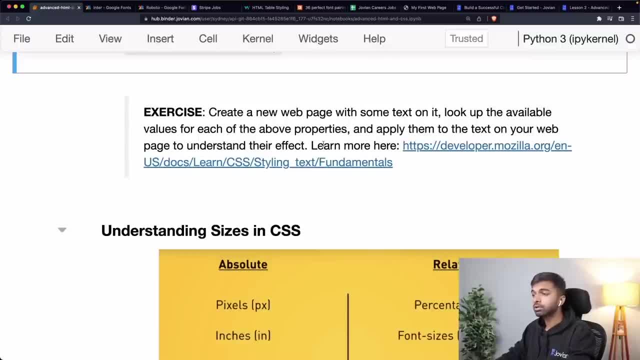 for each of the above properties and then apply them to the text on your webpage and understand the effect. Okay, So the more you practice, the more comfortable you'll get. You don't have to remember this stuff, but you have to know how it works so that when 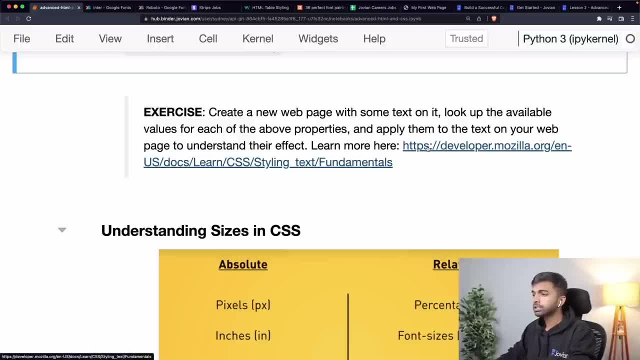 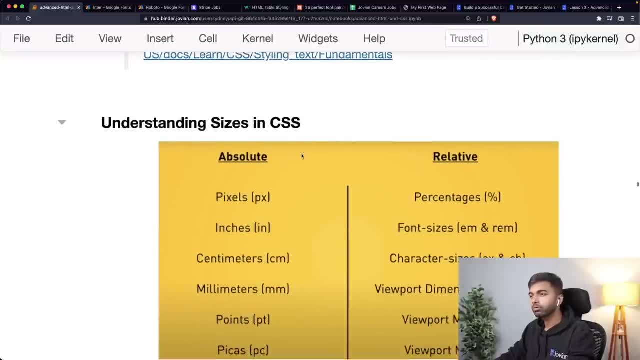 you need to, you can look it up, And there's also this reference that you can check out on styling text. It contains everything that you'll need to know about text styling. Now, one last thing I want to cover before we head into a break. 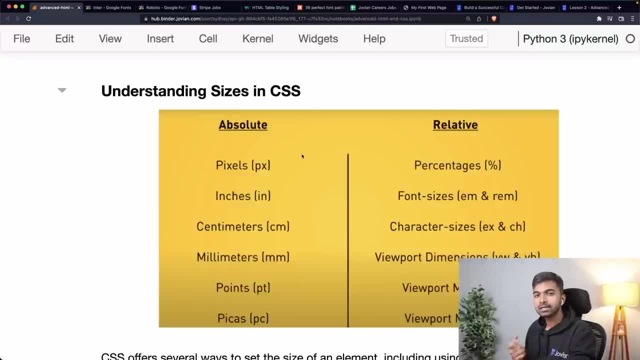 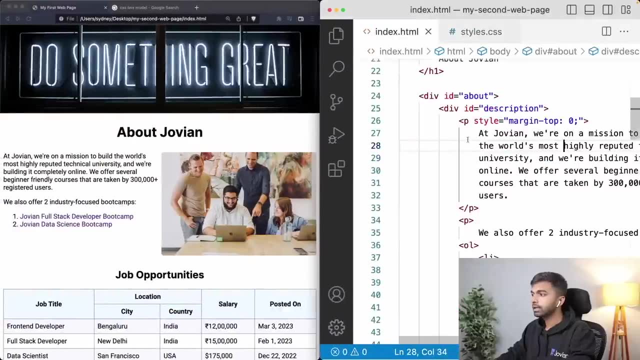 I mentioned to you that one way you can add sizes or lengths in CSS is by using pixels, or another way you can do it, as by using percentages, For example, in index. in our stylescss we have set the max width of the about section. 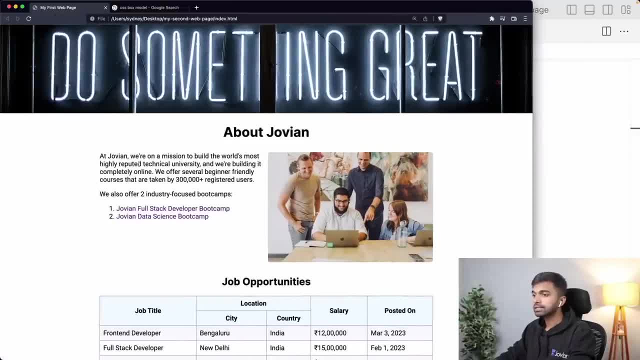 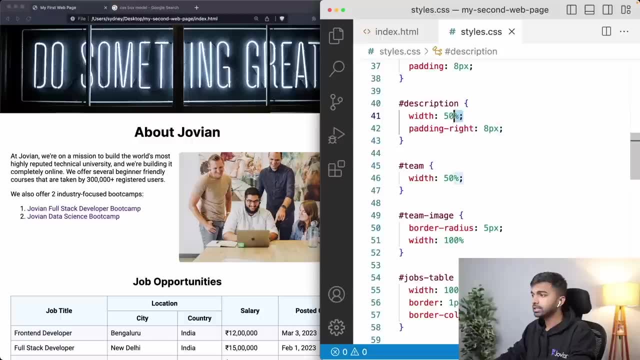 to 800 pixels, And that's it. So, that's it Okay. So it sets the max width of this section, But along with that we can also sell, select a width in percentage. So here we have 50%, which is the weight. 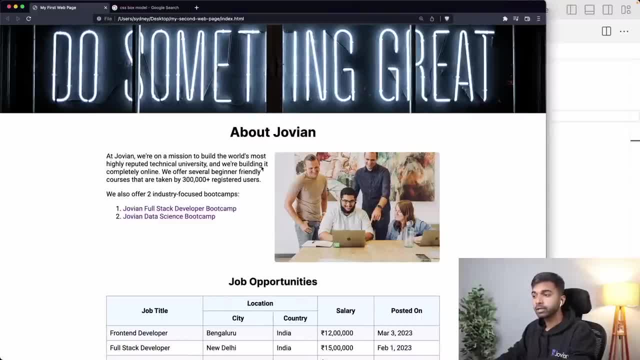 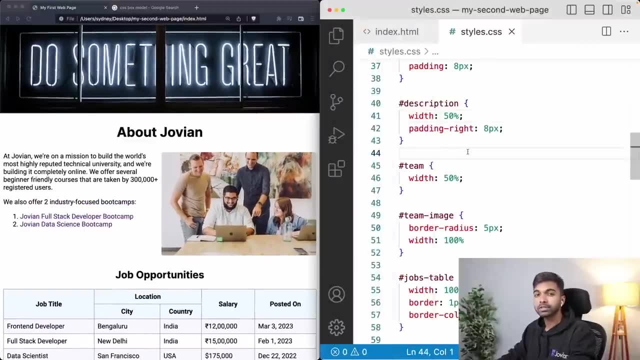 And that ensures that it takes a 50% of its parents with a. so the. there are two kinds of lengths. One is the absolute length, which is expressed in pixels, And then we have the relative length, which is expressed in percentages. 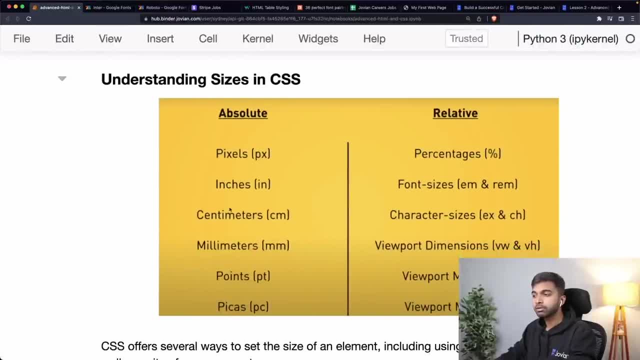 But there are also many other absolute measures that you can use, So you can also use inches, Which corresponds to visual inches on the screen. You can also use centimeters, millimeters, points, or, because all of these are not very common. 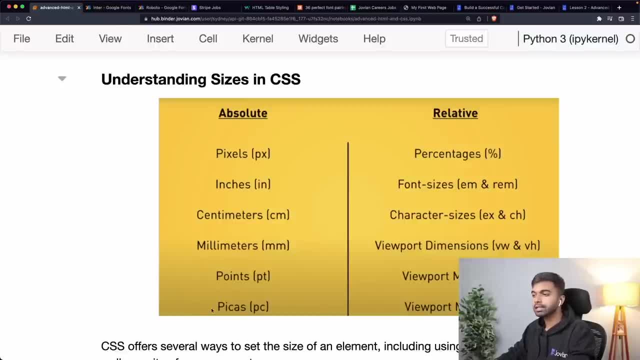 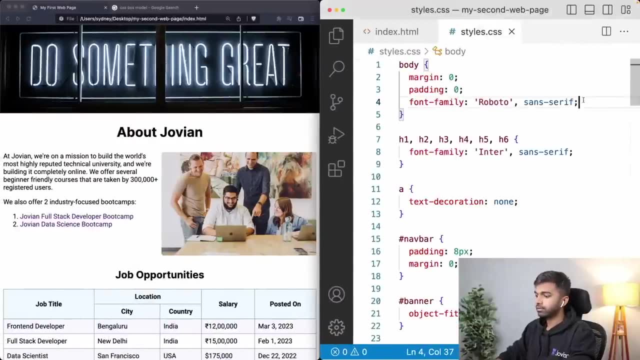 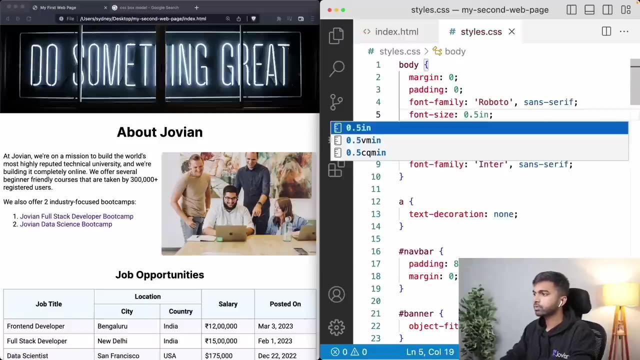 So most of the time you'll only see people using pixels, but just know that these are all also present in case you want to specify it. So let's say we want to set the font size of the body to 0.5 inches. 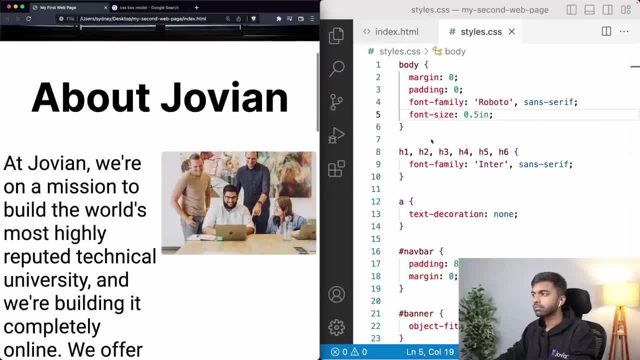 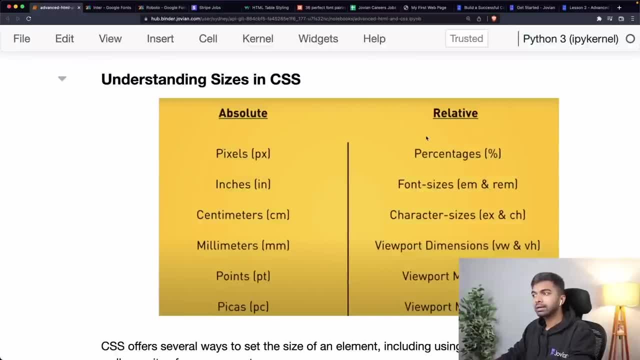 We could do that, Okay, And of course that's very big. We may not actually want that, but that scales the size of the body, Okay, Um, the other thing is in relative font sizing as well. most of the time, you will use percentages. 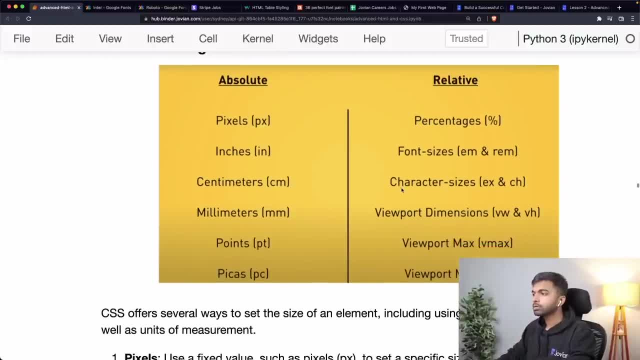 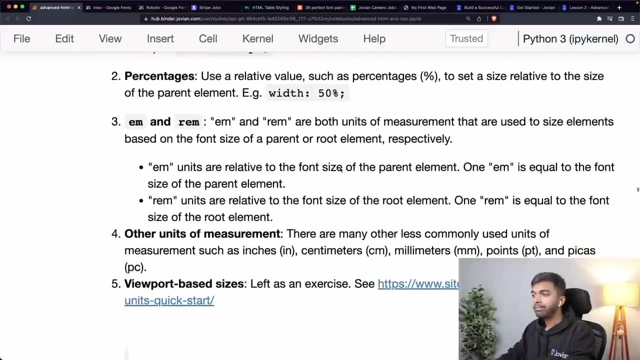 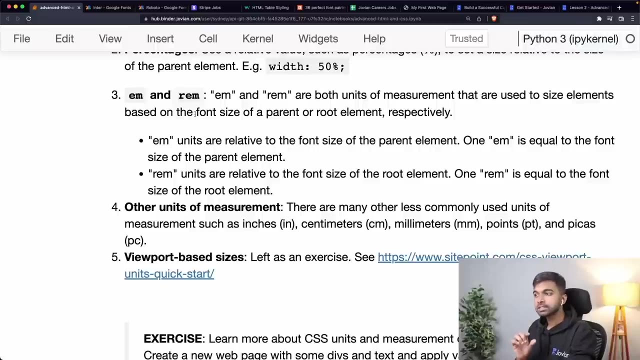 but when it comes to text specifically, people often use these font sizes called EM and REM, M and REM. What do M and REM mean? Well, M and REM are both units of measurement that are used to size elements. Okay, So we're using the font size of either the parent div or the font size of the root element. 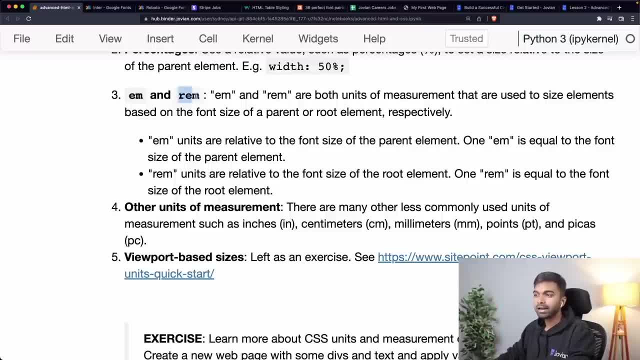 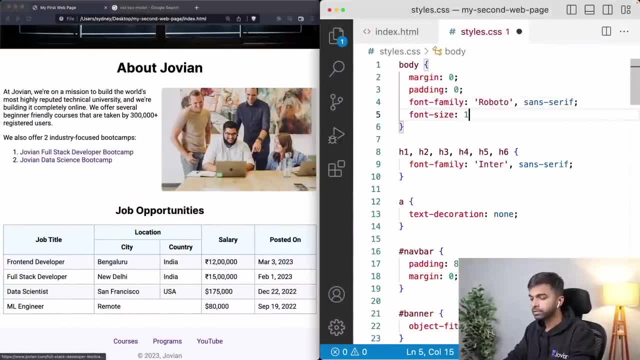 which is the body body tag. Okay, So first I'll tell you about REM. So here's what happens. Let's say I sent a set of font size for the body, font size of 16 PX. Okay, So now I've set the font size of 16 pixels for the body. 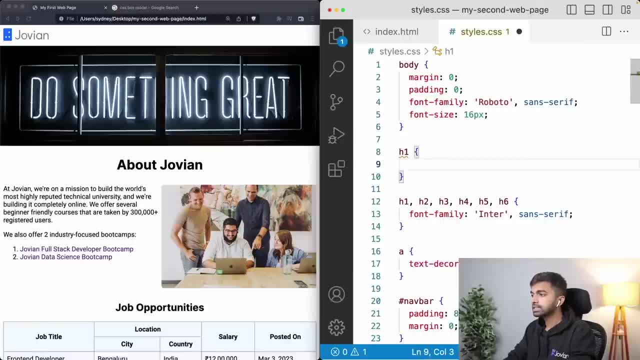 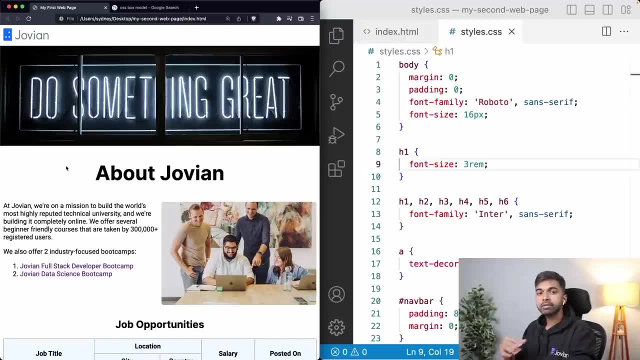 And now let's say I set for each one, I set the font size As Three Rem. Okay, When I set the font size of three REM for H1, what I'm saying is relative to the root tag, which is the body tag. 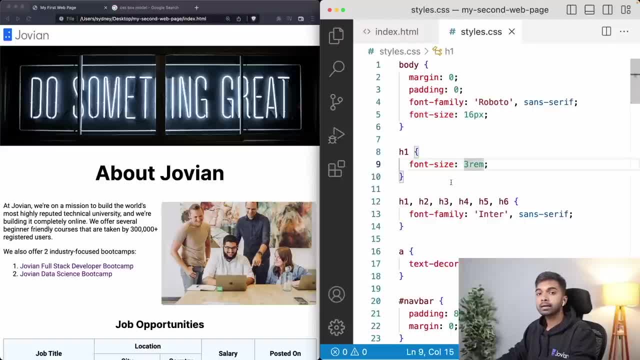 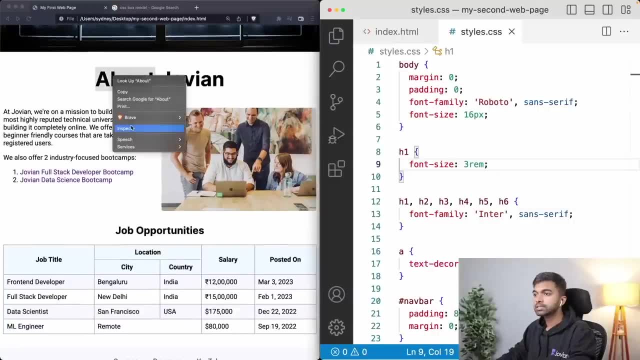 I want the font size of the header H1 to be three X, And that is what is specified by three REM. And you can actually verify this. You can go, you can right click, you can say inspect, and that is going to open up this. 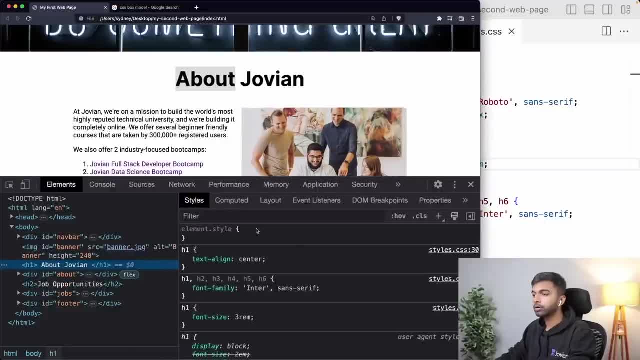 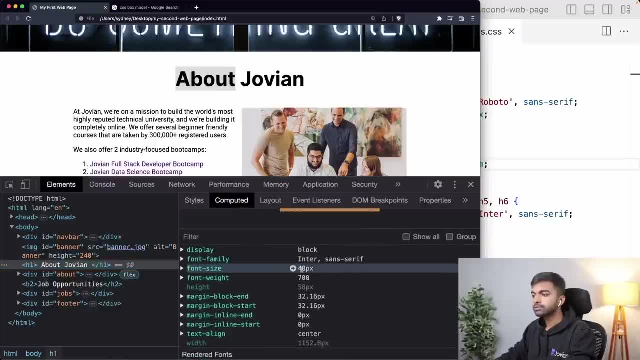 Yeah, So that is going to open up this box model for you. Okay, So you can check this H1 and you can go into computed here and you can verify that it's font size is 48 pixels. So 16 threes is 48, right. 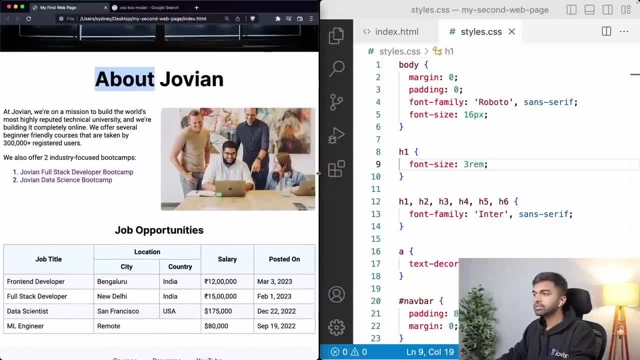 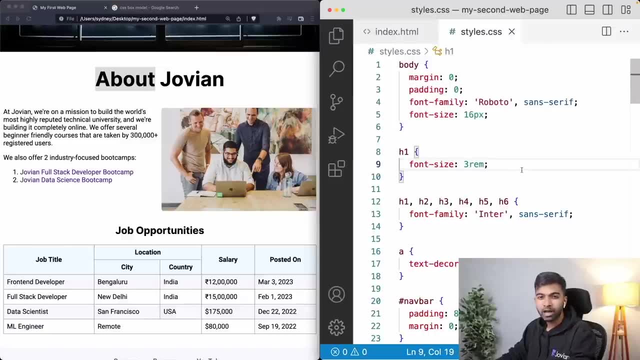 So just by specifying three REM, we have specified that the font size of the heading is supposed to be three times the font size of the body. Why will, why would we want that? Well, why not directly just set it to 48 PX? 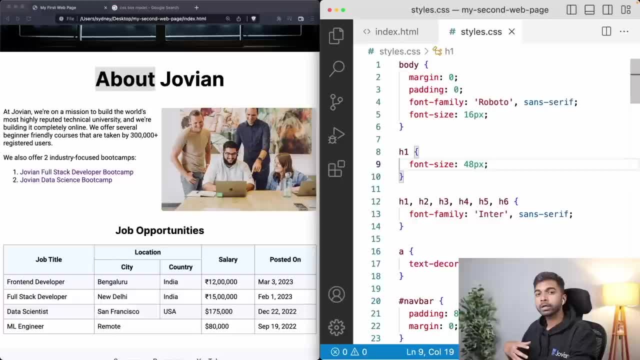 Well, let's say we had a design overhaul and we wanted to change the body font size from- Okay, 16 pixels to 20 pixels. We want to make our text bigger so that people can read it more easily. So if we change it to 20 pixels and reload the page, you can see that the text became. 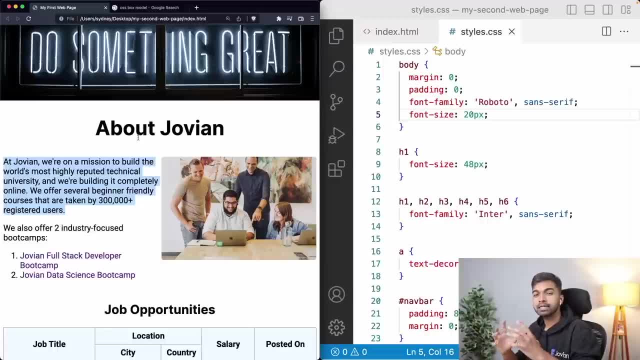 bigger, but the heading did not become bigger. So now we've lost that balance which we had earlier established. On the other hand, if we had three REM here, every time we change the basic- or, yeah, every time we change the basic body size, that is going to. 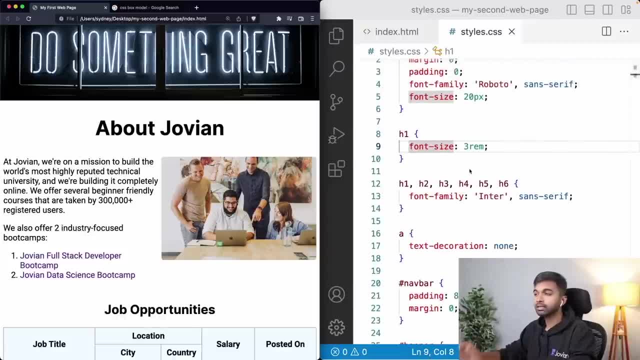 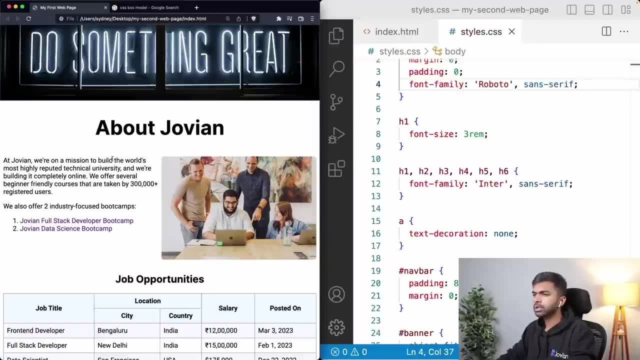 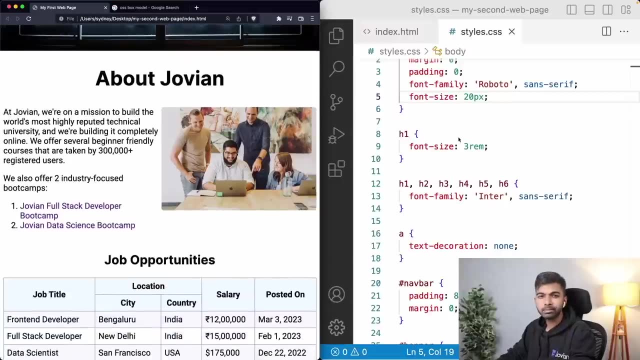 Okay, Yeah, Yeah, That is going to automatically scale the font size of the H1 as well, Okay. So if I remove this, you will notice that the H1,, but it should have become bigger. Okay, There might be something else that is affecting the H1.. 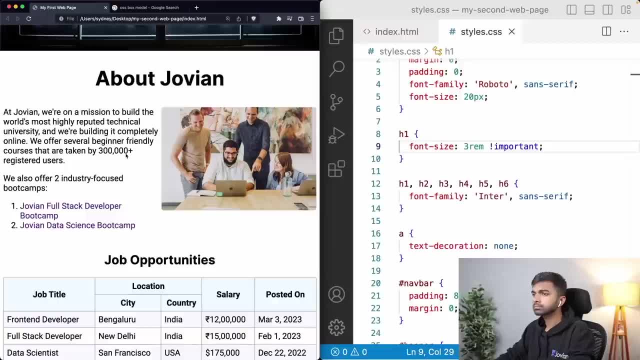 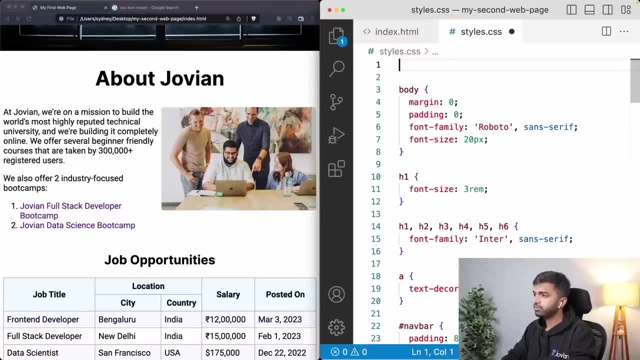 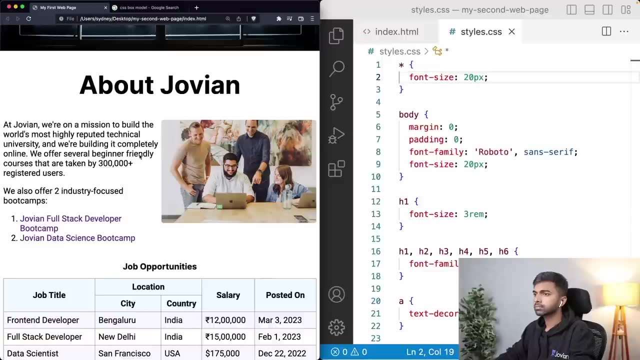 So I'm just going to put in important here. That doesn't do it either. Maybe we have to set it at the root level. Okay, Okay, I will, Yeah, So I believe the root, the root font size, has to be set using star or just using maybe. 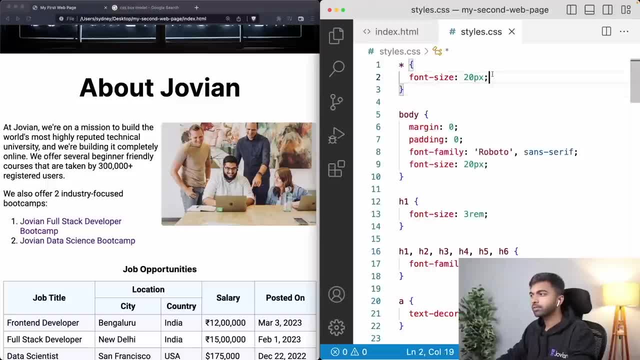 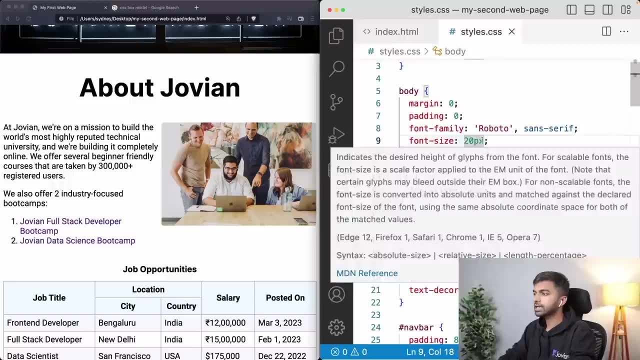 HTML or something. So you said the root or you said the base font size over here using star, and then everything else is expressed as REM of that. So the body font size is going to be one REM And then the H1 font size is going to be three REM. 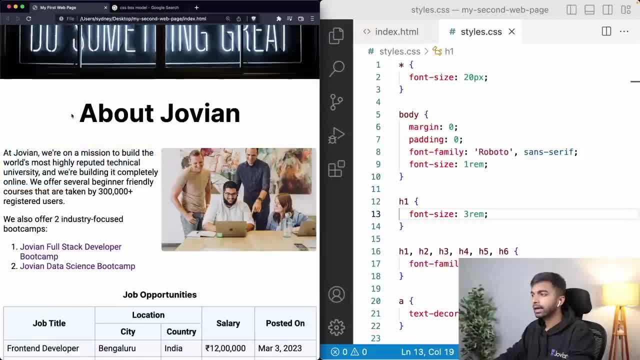 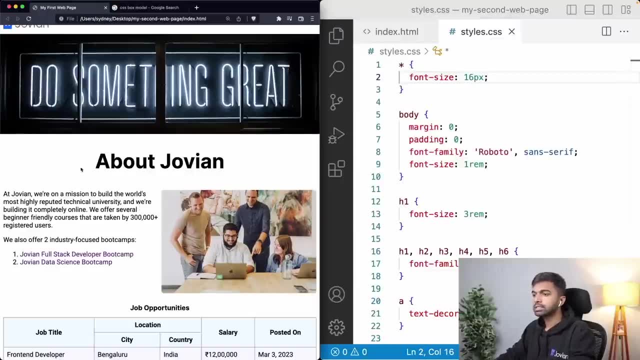 So I if I reload that, you can see that the body is 20 pixels And the H1 is 60 pixels. But if I change the body font size to 16 PX, now you can see that this is a set. 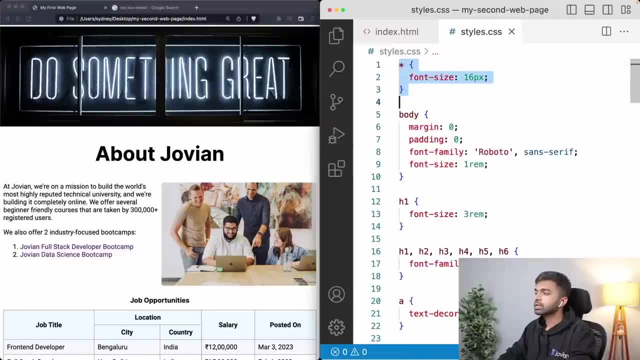 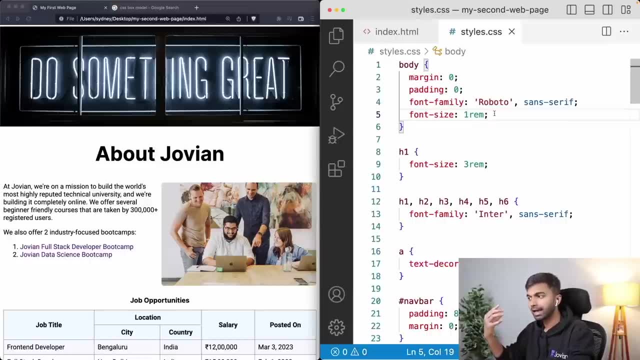 This is now scroll down to about 48 weeks of pixels. Okay, So that is how you use REMS to specify the font size in relation to the root tag of the entire page, But of course, you can also set it to three M, in which case if the H1 is outside another. 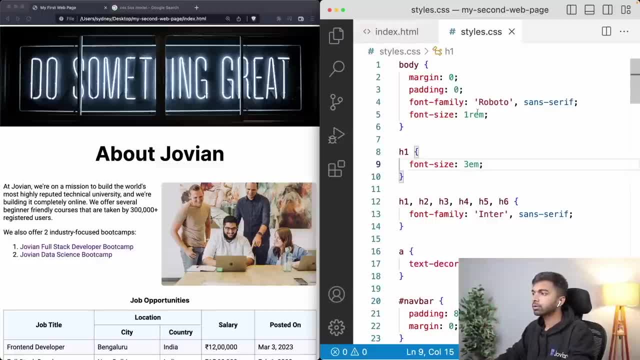 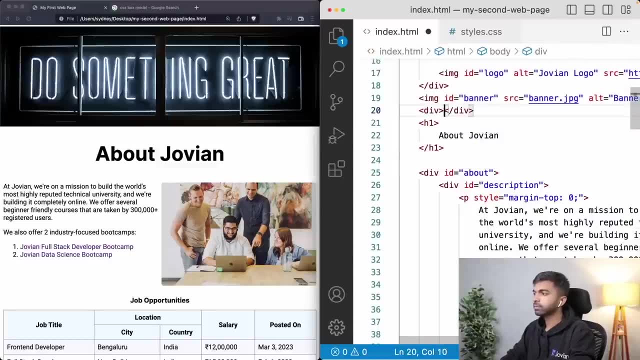 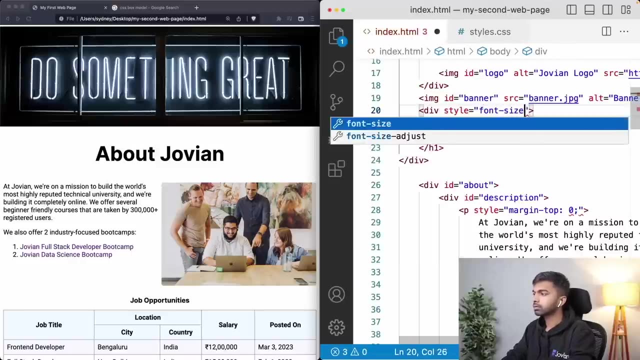 div. If the div has a particular font size, then we are simply going to use the font size, which is three times that. Let me show you an example here. So let's say I have this H1 inside a div and in the div we have set the font size to five. 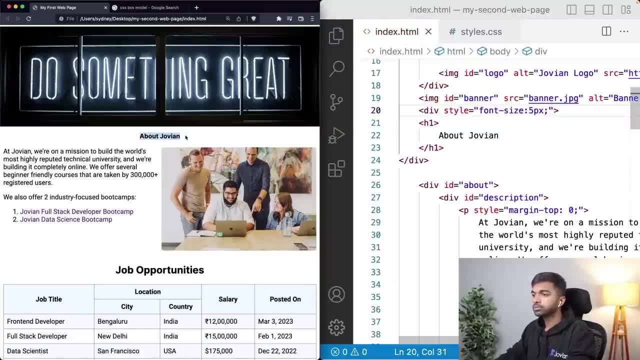 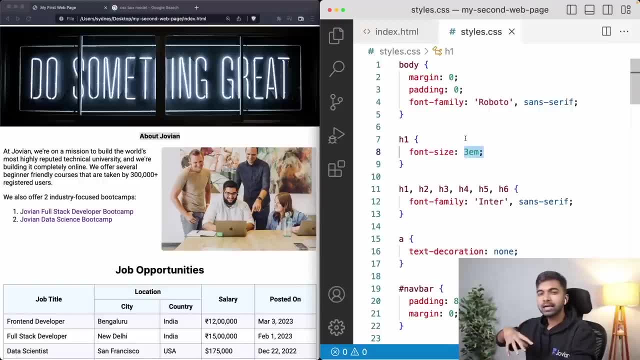 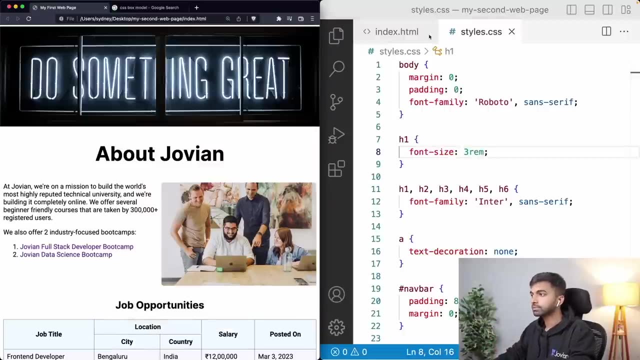 pixels. So now this H1 has the size three times five, 15 pixels, because it is set to three M EM. Okay, So M is relative to the parent's font size, Rem is relative to the default font size of the entire page. 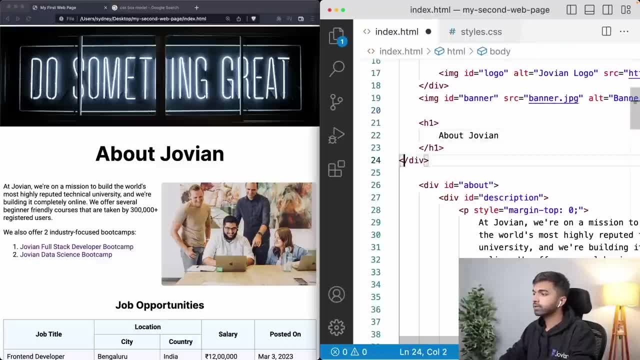 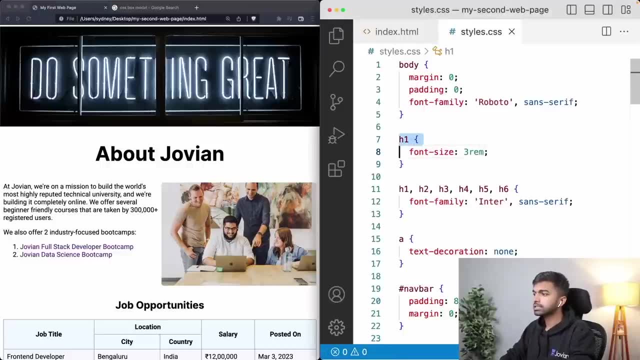 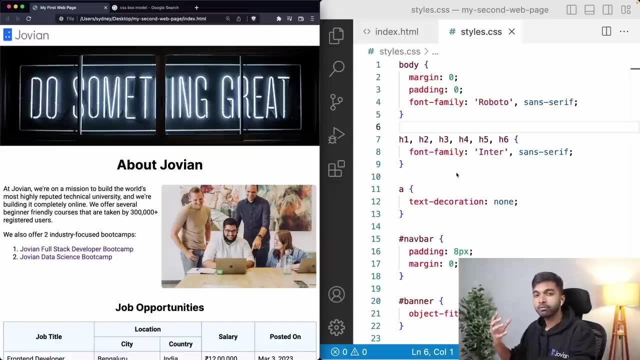 Okay, So that's that. Let us revert that change. So now you might wonder that, since we have all these different kinds of font sizes, how exactly do we decide what font sizes you should be using? How do you decide the font sizes for the different headers? 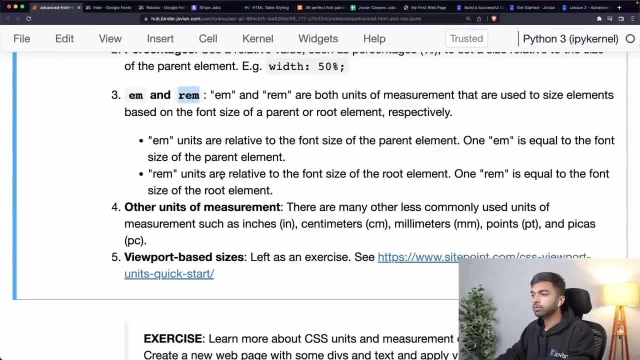 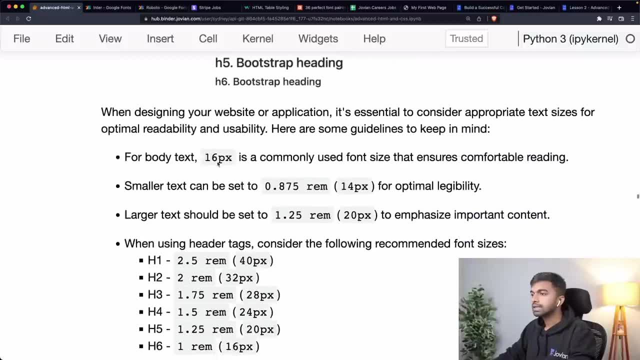 How do you decide the font sizes for paragraphs? So I just want to share a few guidelines for you, Okay, And this is from this library called bootstrap, which we look at in the future. while designing your website, it's important to consider appropriate text sizes for optimal readability and usability. 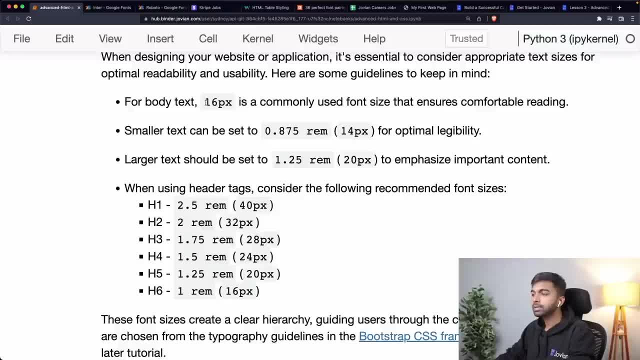 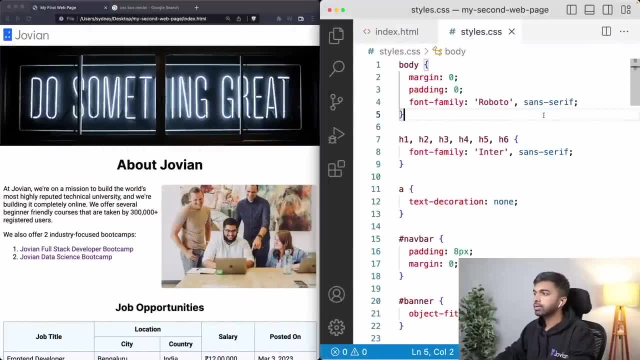 And here are a couple of guidelines. or the body text: 16 pixels is a commonly used font size And this is the default in most browsers. So you can just use that in the body. You can just come in and you, if you just say font size 16 PX, that is going to be. 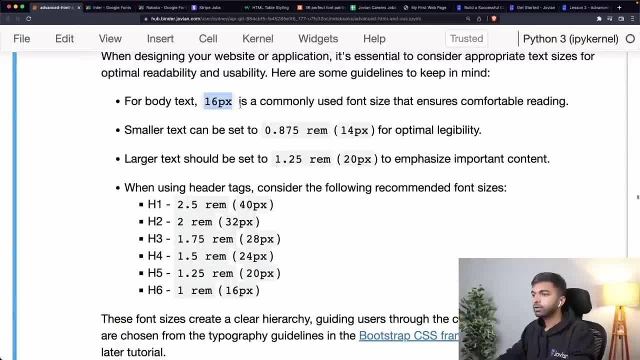 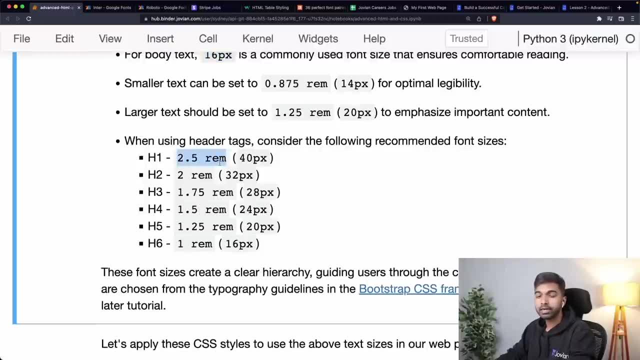 the default font size. You see nothing changes. Then for the headings you can use these font sizes. So for the edge one you can use 2.5 Ram, which is 2.5 times the font size of the body, or 40 pixels for H2.. 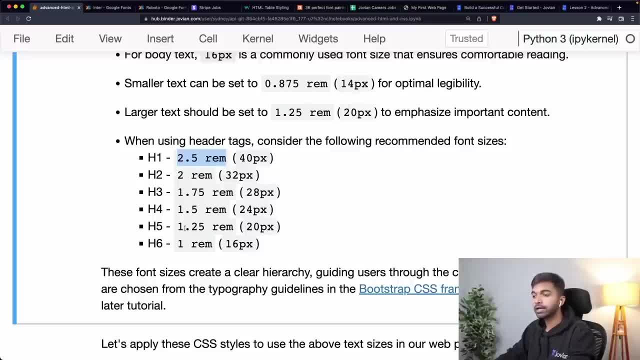 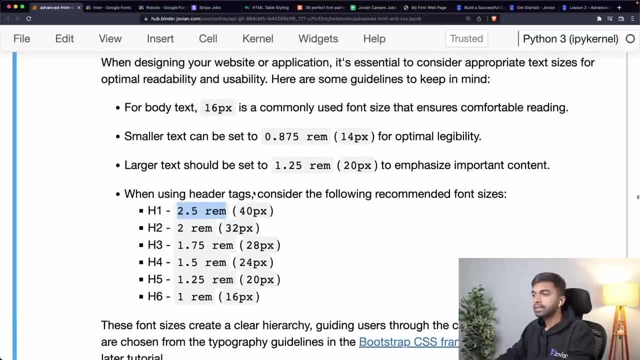 You can use 2 Ram for H3, 1.75,, H4, 1.5, H5, 1.25 and H6, 1 Ram. Okay, And of course all these will also be bold, So you'll have different font weights. 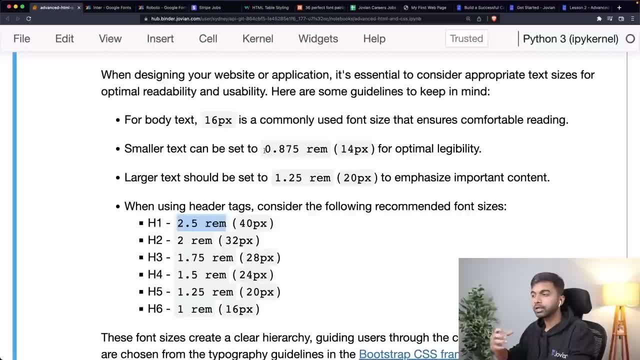 And then if you have maybe slightly smaller text on the page somewhere which is smaller than the body text, Then you can use 0.86.. 0.875 Ram or 14 pixels and any larger text. you can make it 25% bigger. 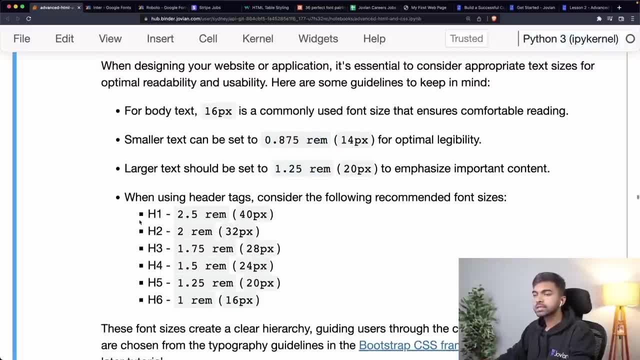 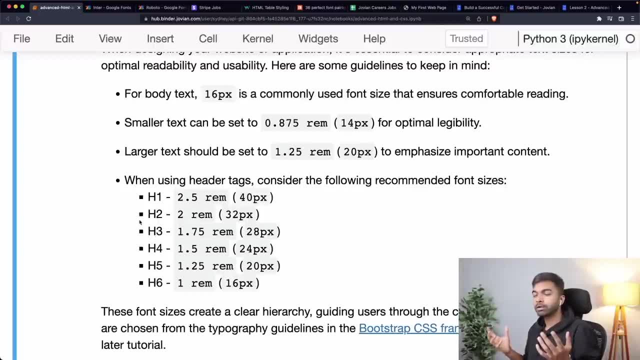 So you can set that to about 1.25 Ram, right? So this is a good rule of thumb that you can have. Nobody tells you this when you're learning HTML, but it's very difficult to determine what font sizes you should have. 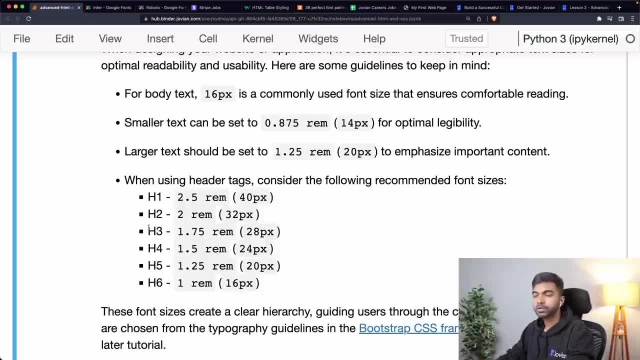 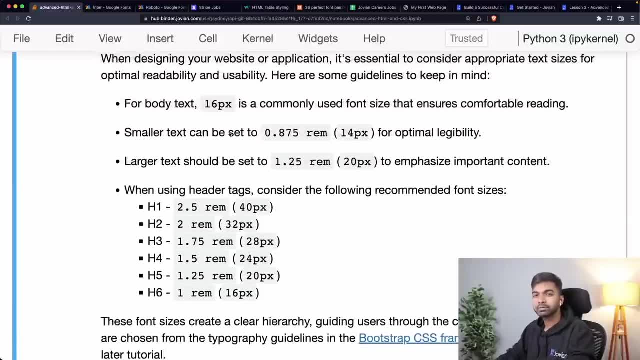 So just use this, keep the screenshot with you, And most of the time you'll be using a library, So this won't be a problem. but if you're working at a company, you'll probably have a design guide which will specify something similar for you. 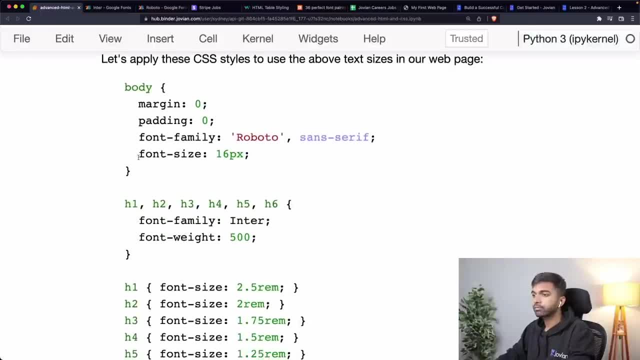 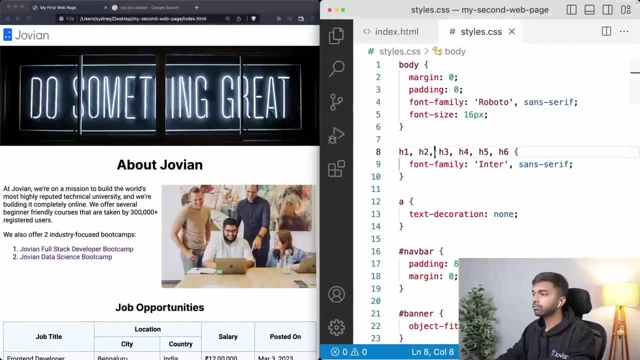 As well. Okay, So let's apply these font sizes. So for the body, we have the font size of 16 pixels for H1 to H6.. I'm going to use the inter font and I'm going to use the font weight of 500 as well. 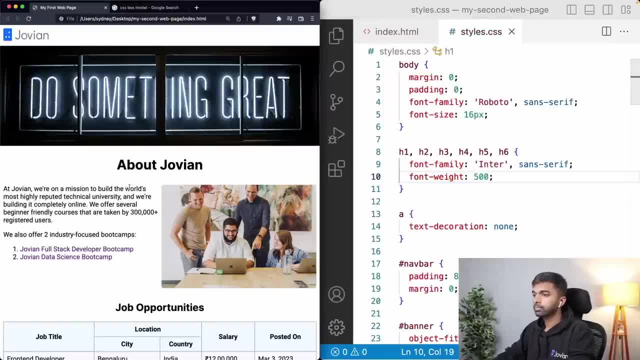 So font weight: 500.. So I just want to make it a little thinner, I don't want it to be so thick, or maybe 600.. Let's see, Yeah, I think I like 600, so I'll keep 600. 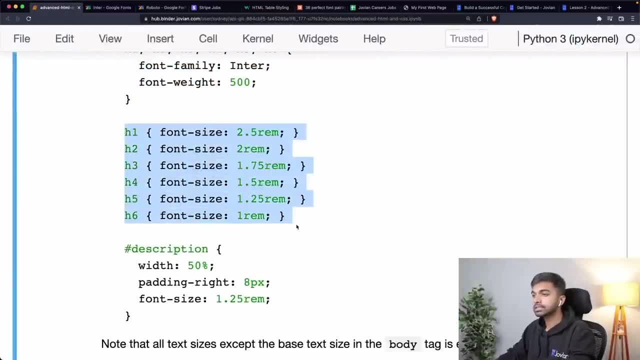 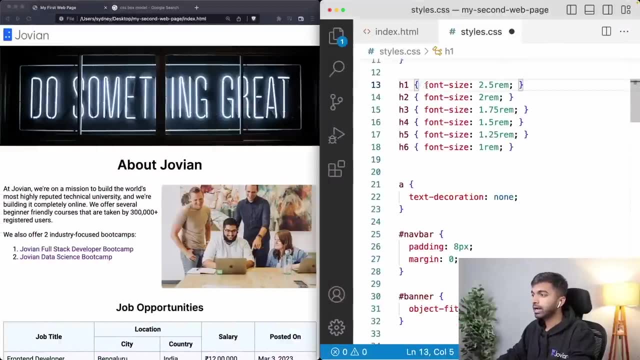 And then I also want to set the font sizes for H1 to H6.. Okay, Okay, So let us set the font sizes for H1 to H6 again. I am just selecting the H1 tag, opening this bracket, putting in the, putting in the property font size and then using REM. so 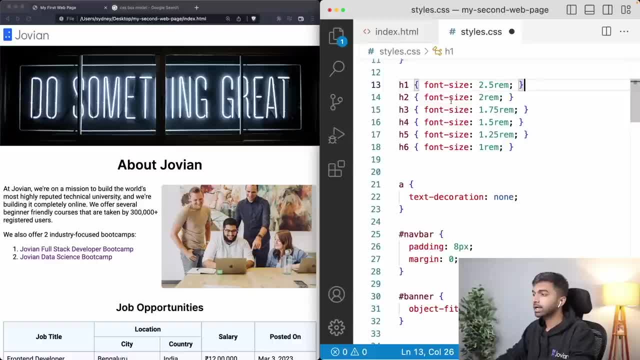 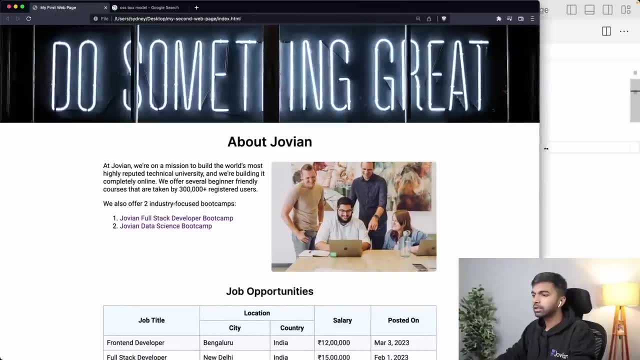 that if we change the base font size of the page, all of the scales automatically, So 2.5 to one REM for H1 to H6, and that's good. And one other thing I want to do is this particular section over here. I want to make it a little. 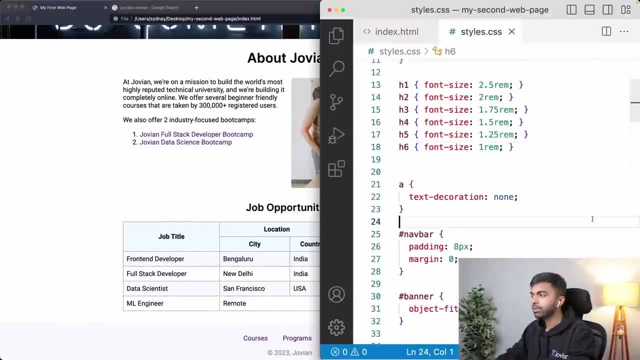 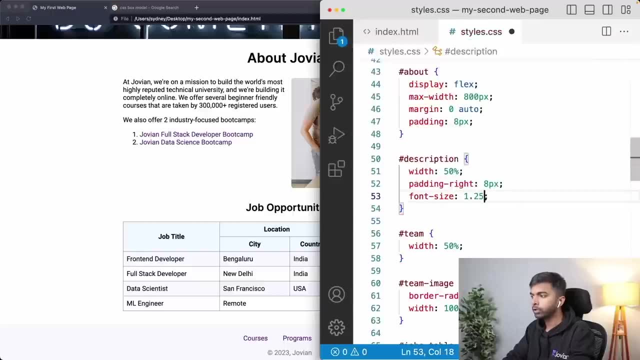 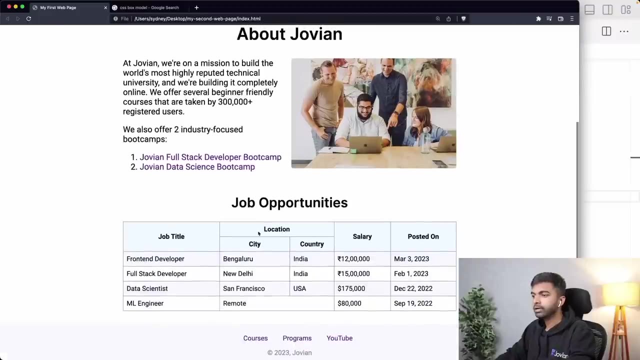 bigger, so that it's bigger than the rest of the text on the page. So I'm going to come in here into the description section and I'm going to say font size: 1.25 REM. And now this is a little bigger, a little nicer, all right, compared to this table. for instance, or compared to the footer, And of course I could go in here and I could make this smaller. So I could come in here into the copyright and I could say: font size: 0.875 REM. Okay, Now it is slightly smaller. 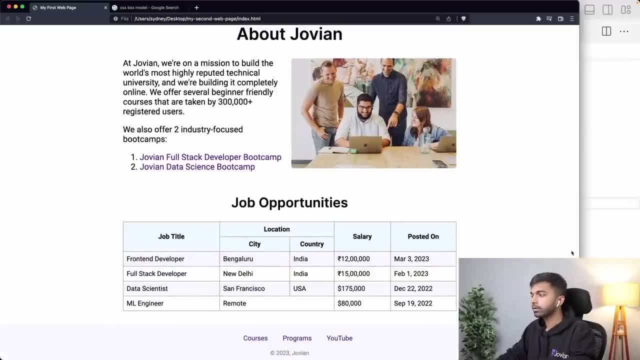 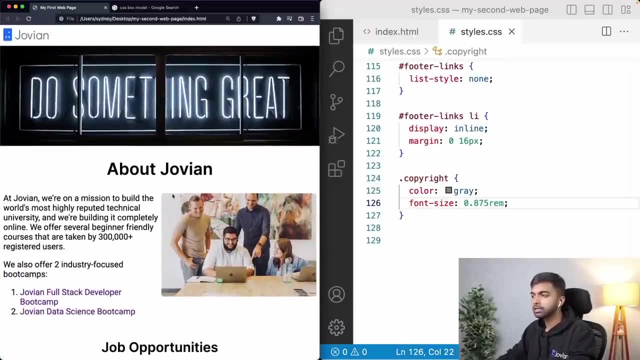 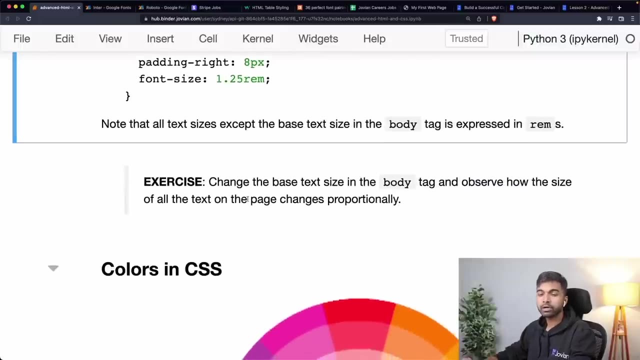 Okay, It is slightly smaller than the rest of the text right, So at page is already starting to look aesthetically a little nicer. We have these font sizes. The next thing we should probably fix is the colors. We have too many colors on the page, but that is how you set sizes for text. 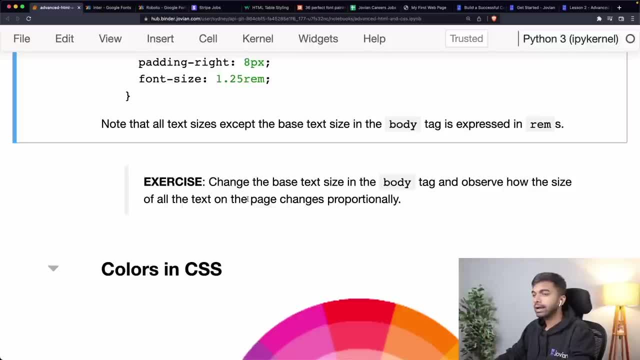 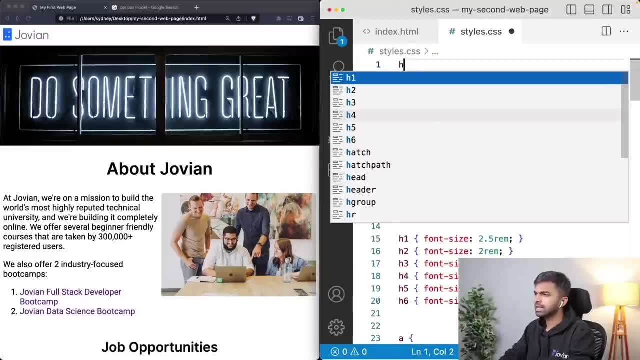 That is how you style text in various using various properties And as an exercise, you can try changing the base text size. I believe you can just go in here and you can select the HTML tag and say font Size: 20px. 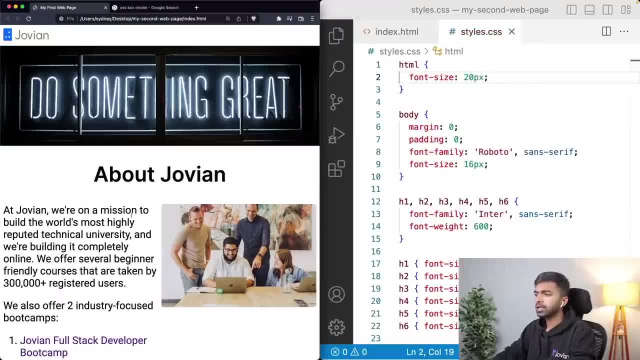 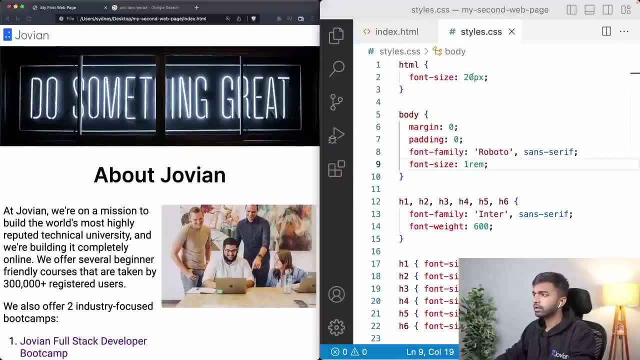 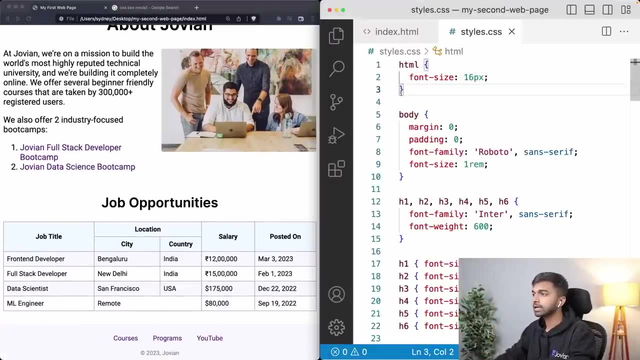 And I think we should make everything bigger. You can just put body as one REM as well, So yeah, And if you come back, make this smaller, everything becomes smaller. So that's how you can scale for font sizes up and down for the entire page: by just setting. 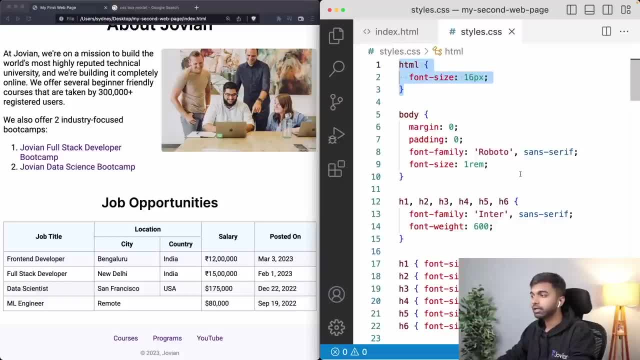 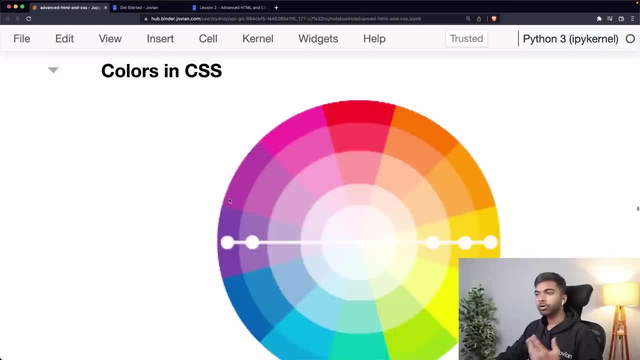 it up on the HTML tag and then using REMs everywhere, or even M's in some cases. Now let's talk about colors in CSS, because this is where a lot of people face a difficulty. I'm going to show you how to do that. 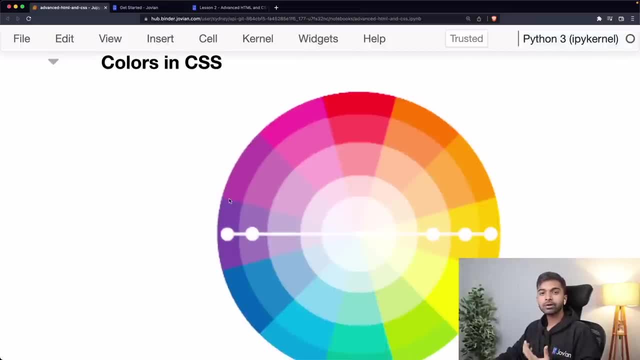 Okay, Let's talk about color. What color should I put? Why is my webpage not looking good? The single reason, the number one reason why web pages often look ugly is because of poor choices of colors and contrast. That's why we have a dedicated section. 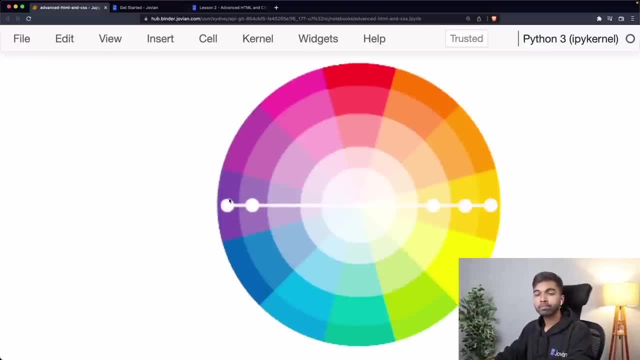 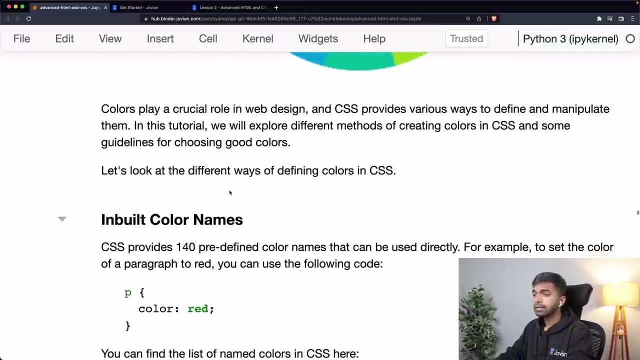 And again, this is not something that we, that people, go into in an introductory HTML and CSS lesson, but we want to make sure that you build good, visually appealing web pages. That's why we're talking about color And colors. colors play a crucial role in web design and colors also convey brand colors. 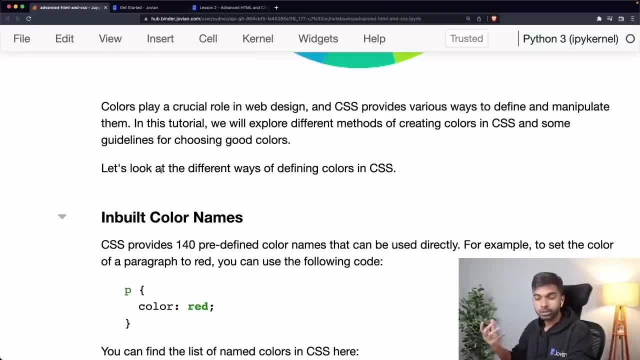 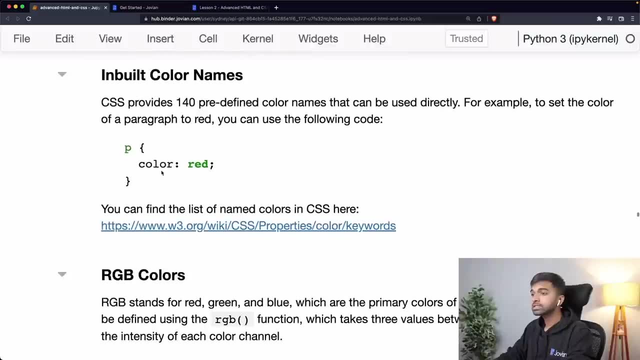 also convey balance. Colors also convey emotion in a lot of cases, And there are many ways to incorporate colors into your web pages using CSS, And the simplest is, of course, using the inbuilt color names. So CSS provides 140 predefined color names that you can use directly. 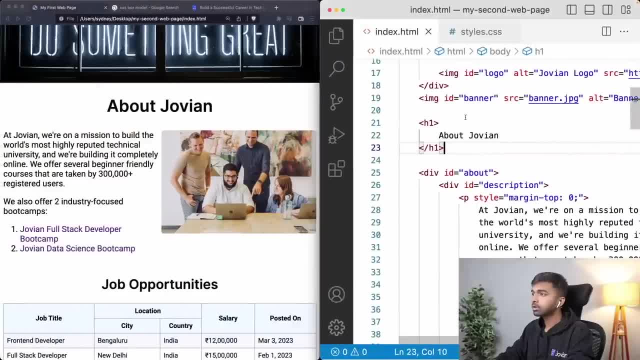 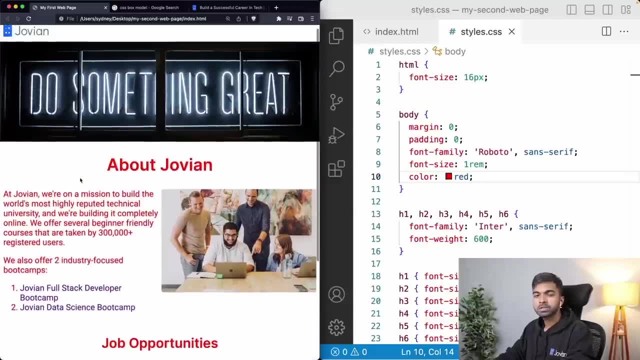 For example, you can set the color of a paragraph of text to red. So I could come in here and I could say color red, and that would make all the text on the page red, which is obviously not very nice. But when you're starting out you tend to pick some of these basic colors. 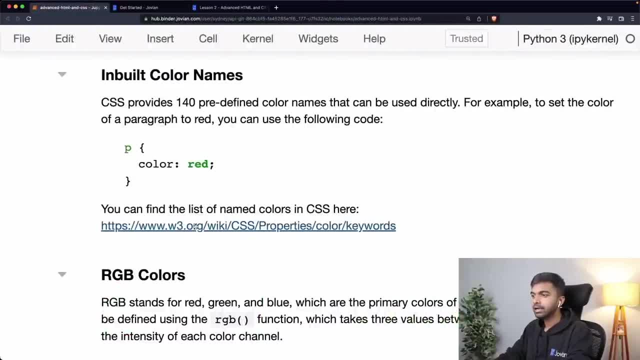 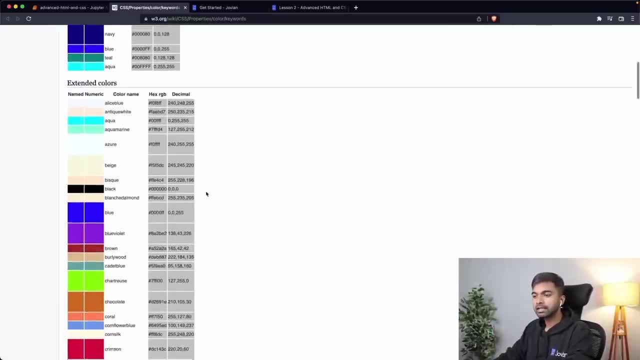 Don't use them. They look at they make your page look bad. instead, If you have to use named colors, if you're not sure what colors to use, pick some slightly muted colors, slightly pastel or softer colors. So you could use black or you could use gray. 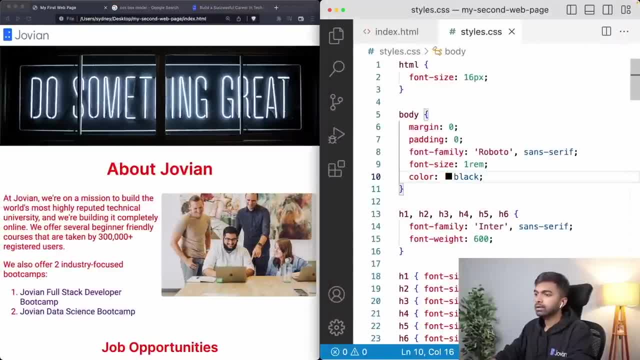 Most of the text on your page should be some version of black or maybe some shade of gray. Sometimes you may have a slight tinge of blue or a slight tinge of some other color, but definitely not. It should be a strong color of any kind. 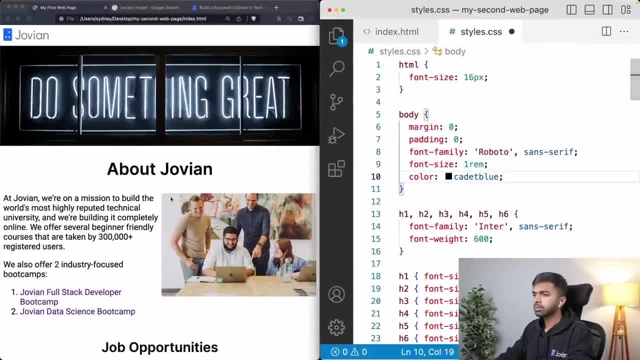 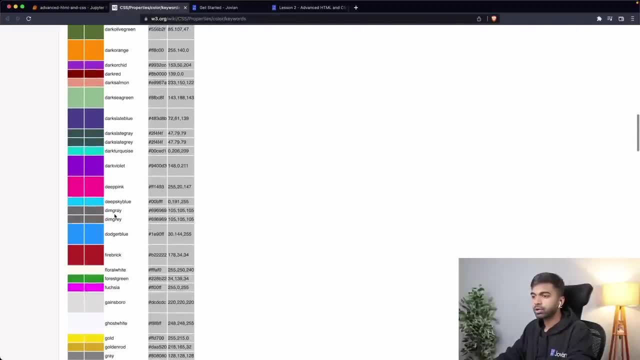 For example, this one cadet blue is an interesting color So I could probably use this. This could be a nice color to use. Okay, Still too different, Probably not that great, So I should probably just use one of these grayish colors, like dim gray. 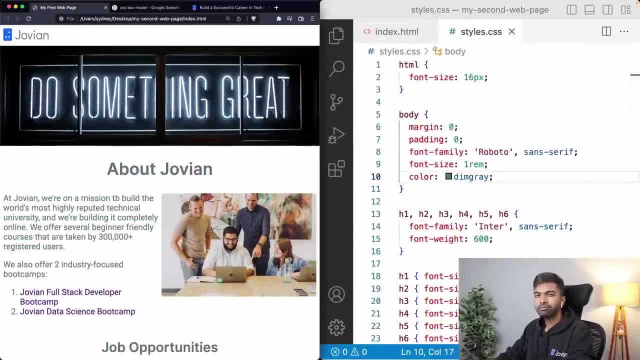 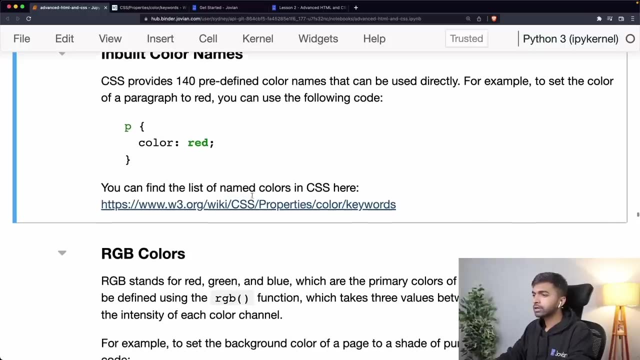 Let me just come in and use dim gray, And dim gray definitely looks somewhat nicer, but it's still not better than the default. Anytime your color choice is not better than default, it's probably a poor choice, But you do have 140 plus choices of colors that you can pick. 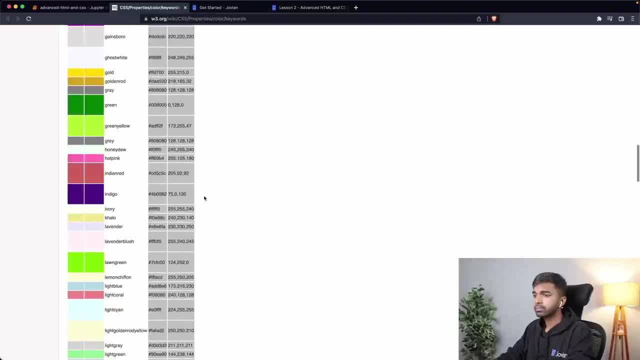 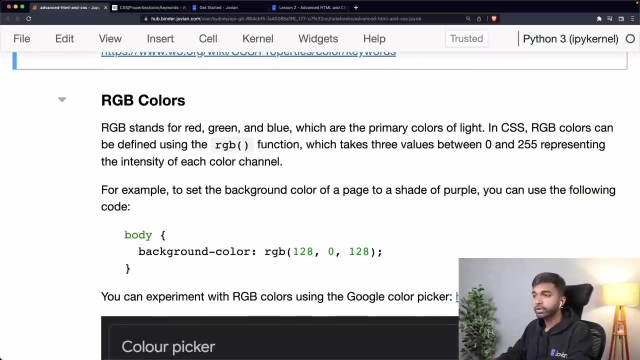 And these are all named colors within CSS. Okay, Next, you have colors that you can define using the RGB system. So RGB stands for the red, green, blue, which are the primary colors of light. So all the colors that you see around you, all the colors that you see on the screen. 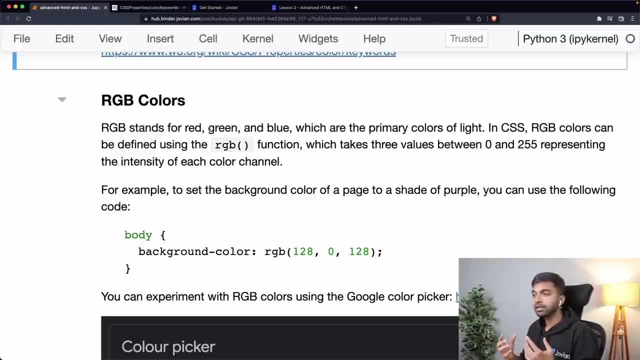 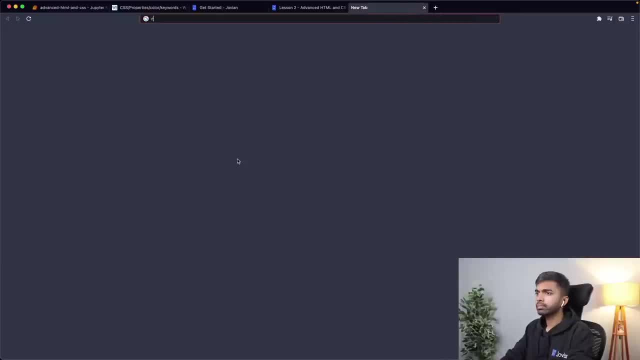 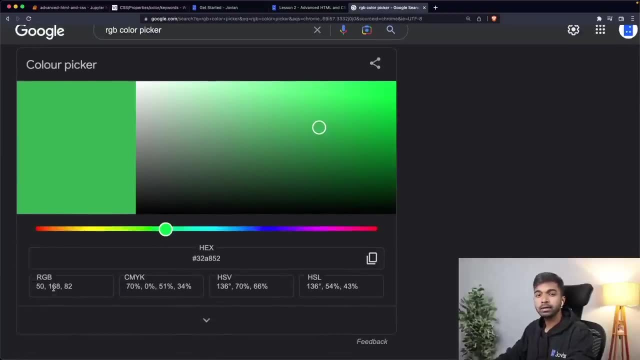 specifically, are built using combinations of red, green and blue. What you can do is there is this RGB color picker here. I'm just going to search RGB color picker. It's a bill inbuilt color picker in Google And into this color picker you can color picker. 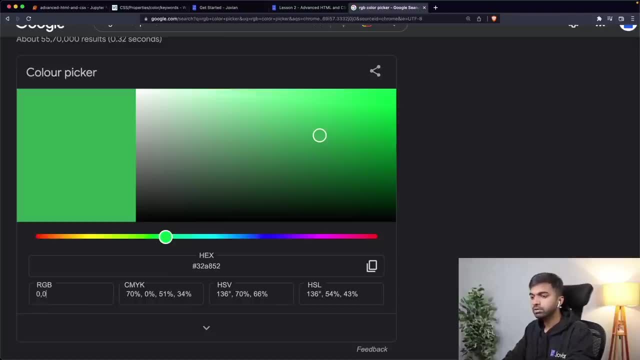 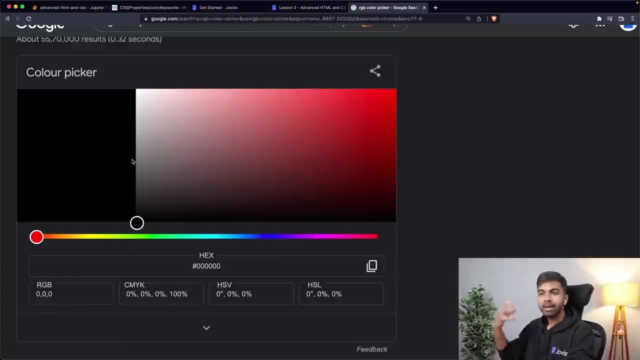 You can select a value for red, green and blue. Let me put zero, zero, zero and press enter. So when you have all of them set to zero- red, green and blue all set to zero- then you get the color black, which means you have no red, no green, no blue. 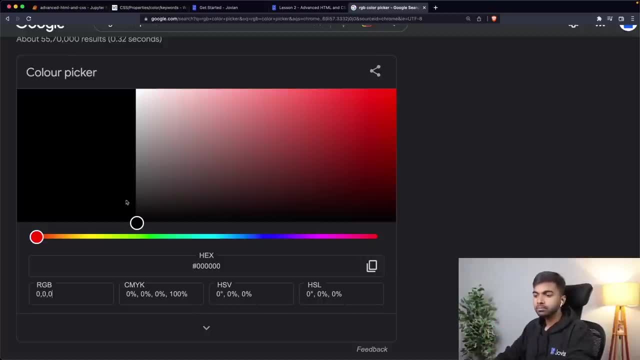 Okay, Okay, No blue, Everything is black. On the other hand, let's say I start increasing red. I increase red to 10. It starts to get slightly redder. I increase red to maybe 40. It's getting more red. 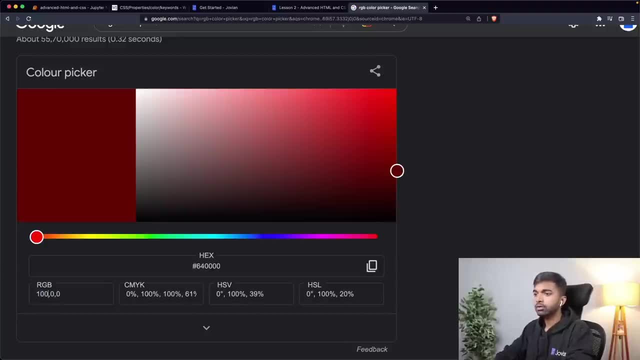 I increase red to 50.. Okay, More red. I increase red to a hundred. Now it's like a dark red. I increase red to 200.. Now it's a very bright red. 150, red of 150 would be something in between. 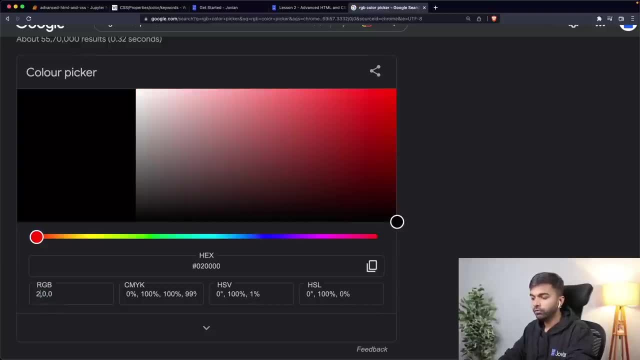 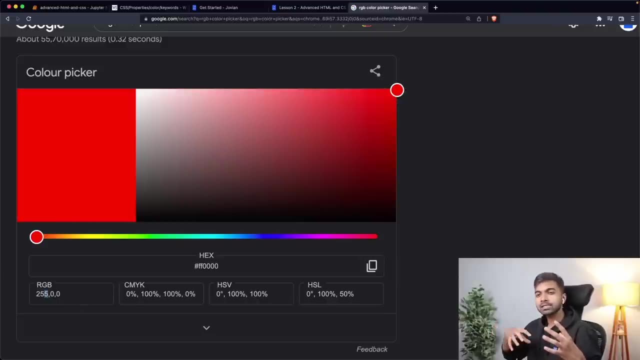 Now it's a medium red And maybe somewhere right at 255. It's the brightest red. Now you cannot have values higher than 255.. So because of how colors are represented internally in the computer memory, you have to choose values from zero to 255. 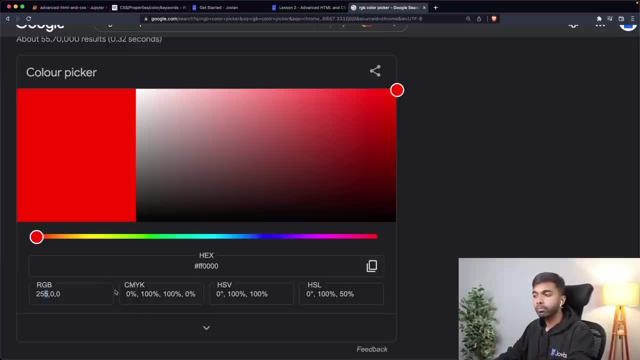 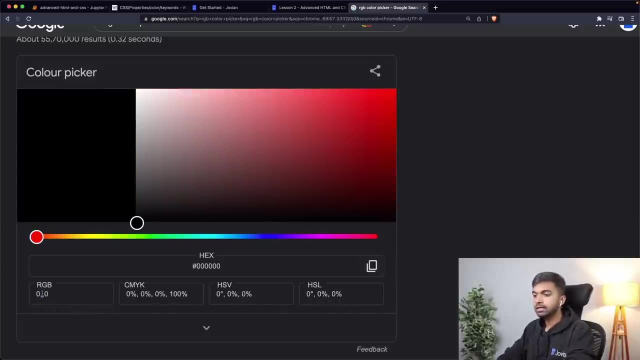 Zero is the darkest and 255 is the highest or brightest, And of course that is the color for red. You could do a similar thing with green. So let me set red to zero, Let me set green to 50, and now you're getting a dark green. 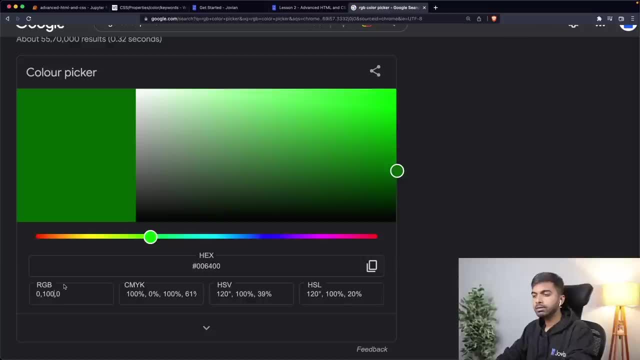 Let me set green to a hundred, and now you're getting a darker green, a slightly brighter green. Let me set green to 150.. It's starting to look light. Let me set green to 255.. And now this is the brightest possible green that your computer screen can display. 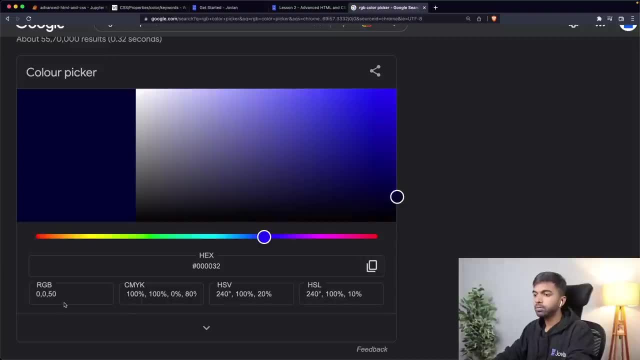 Similarly, we have blue, So this is the 50 blue, This is the hundred blue, This is the one 150 blue And this is the 255 blue. 255 is the brightest, zero is the darkest. Now, of course, you can combine. 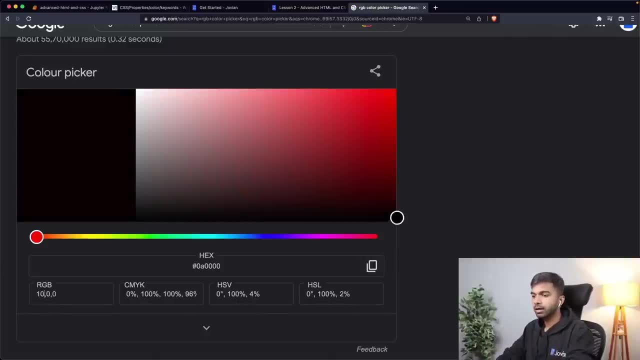 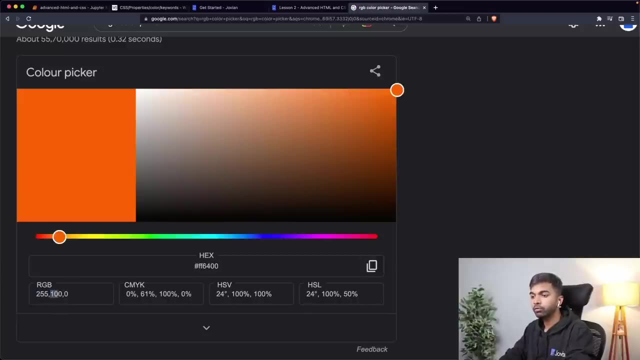 So you know that red and green, when combined, become yellow. So you can say 100 and 100 and that gives you a yellow ish color, but it's still not completely yellow. You have to go all the way to 255 and 255 to get a proper yellow color. 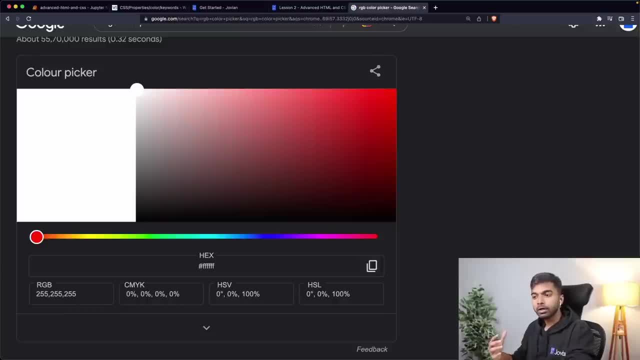 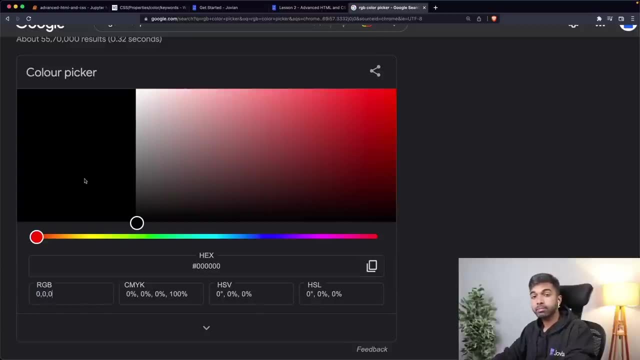 Right, And if you combine all three colors in equal quantity, you get shades of gray. So 255, 255, 255 is white and 0 0, 0 is black. Of course, somewhere in between, let's say a hundred, a hundred, a hundred is going to. 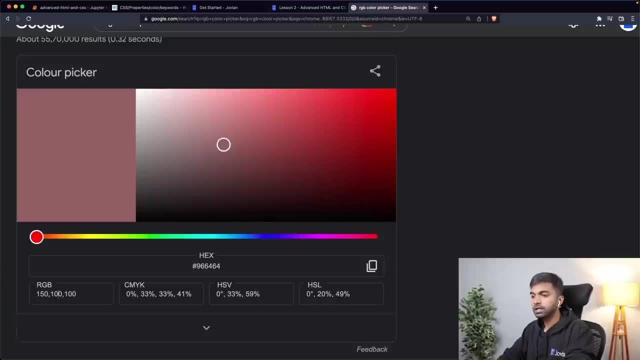 be gray, And you can make this gray lighter By going 150,, 150,, 150, and you can get all different shades of colors by combining various amounts of red, various amounts of red, green and blue, For example. I believe green and blue together give you the cyan color and then red and blue. 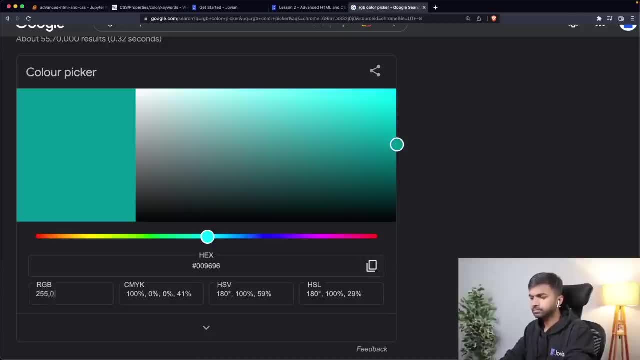 together. Give you- I don't know what it is, Let's see- red and blue together. give you the magenta color, right, So you have all these other colors that come together as well. Of course, you don't have to type out all these colors directly. 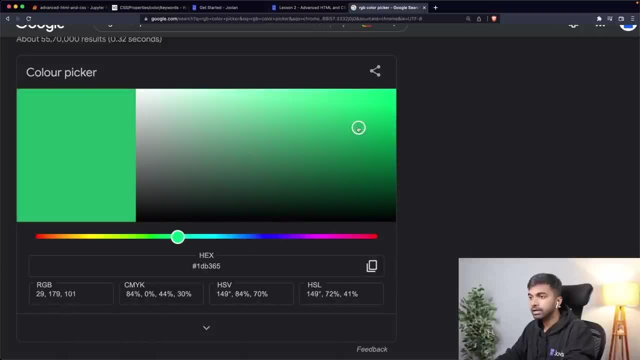 Sometimes you have. you can work the other way. You can go and select a color here That seems nice. Okay, Maybe this color seems nice, I'm going to use it. I'm going to use it for some of the text. not a great color for text, but let me just 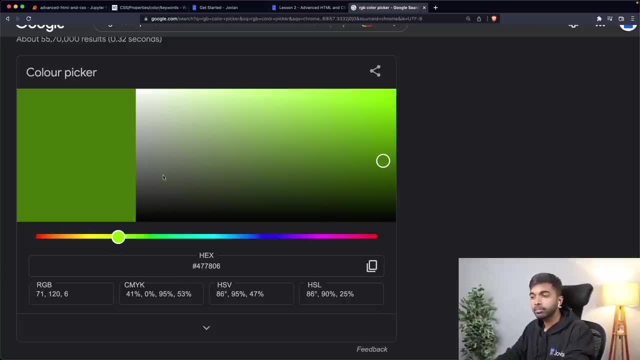 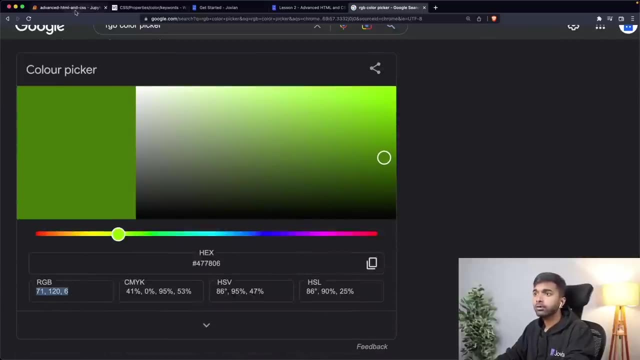 try using it anyway. Then I can just select that using a color picker and you can just search color picker on Google and get this widget and I can copy these red, green and blue values. Now we can come back into my webpage and let me just change the fonts. font color for now. 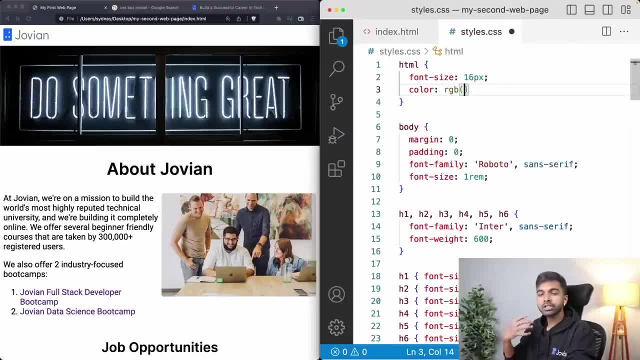 So color RGB. So we use the RGB function and then paste the red, green and blue value And that will just apply the color to that particular element, whatever is selected. right now I've selected the entire page. That's why it's applying to the entire page. 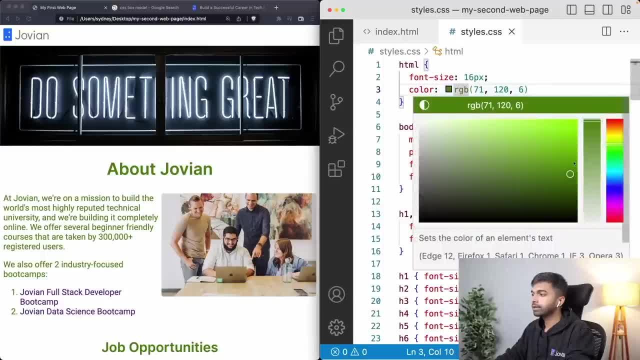 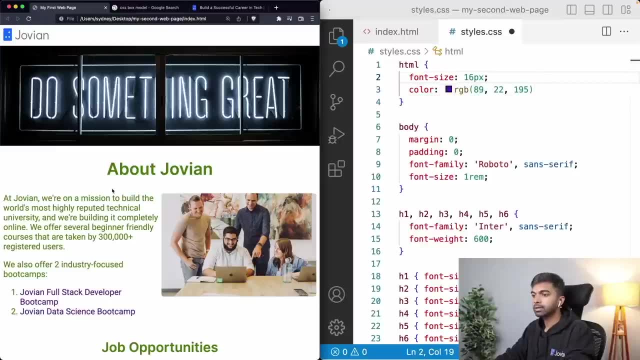 And now I can modify. this VS code actually gives you a color picker directly over here. You can actually go in and select a value directly from here and that's going to modify it And you can then use that color on your page. Oh sorry. 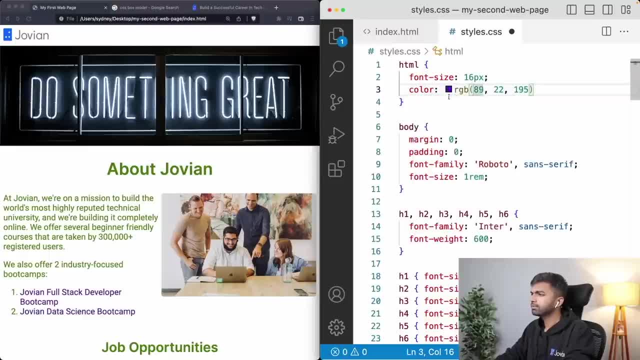 You have to. You'll have to copy it And I believe then you can use that color on the beach. So there are ways to do this within us VS code itself. but whatever red, green, blue color combination you have, you can use that. 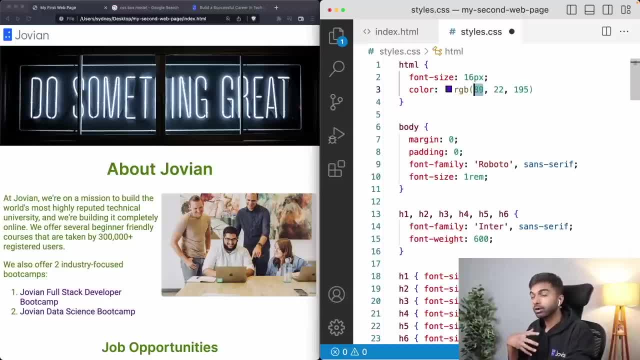 And for now let's just set the default size to some, or the default color to a gray, not exactly black. Let's set it to maybe 210, 210 and 210, maybe a slight tinge of blue, maybe set that to. 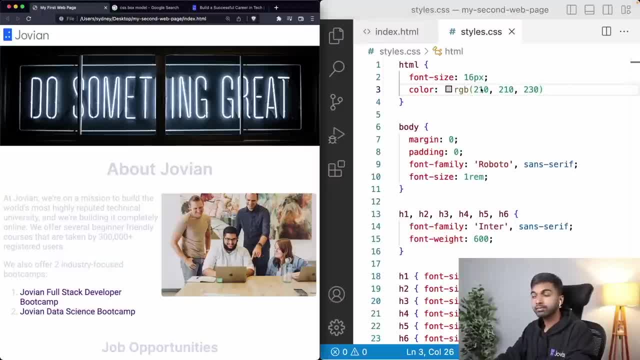 230.. Okay, That's actually very light. So maybe let's make it very light, So maybe 30,, 30, and maybe 40 over here, Yeah, And that is looking actually not bad, Right? So zero is dark. 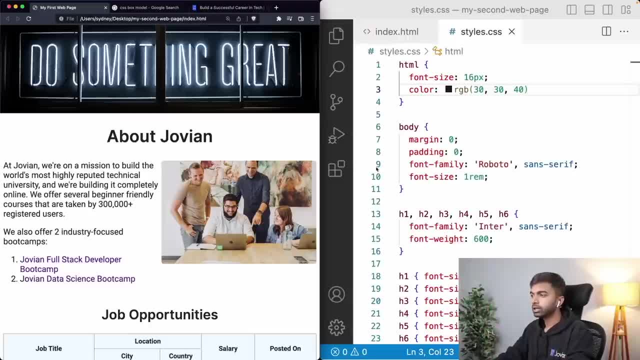 Who 55 is bright and combined red, green and blue. Okay, So that is the RGB system. You can use the RGB function. You can use it for background colors. Let's say, I want to use it not for the color of the page but for the background color. 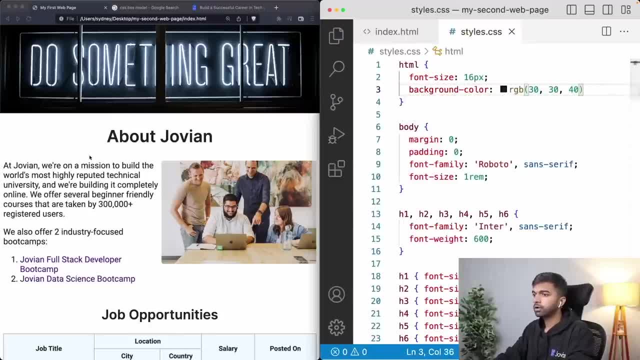 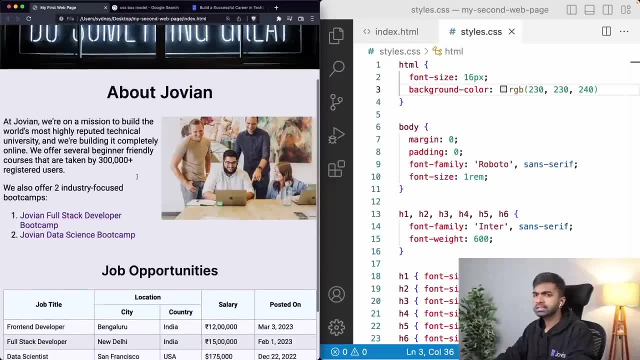 background color of 30. Okay, 30,, 40, 40. That's very dark. Maybe let's set it to 230, 230, 240.. Yeah, that's a fair background, but generally speaking, even backgrounds, it's okay to just. 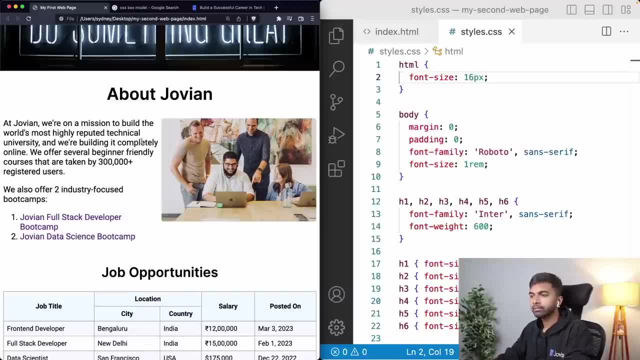 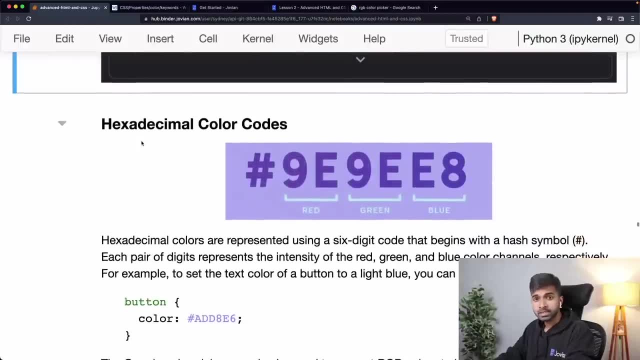 keep them completely white, or a very, very light play, or very, very light gray. Okay, So that is the color. Then there is another way to represent colors, which is using the hexadecimal color codes. Okay, So the hexadecimal is a textual representation of all colors. 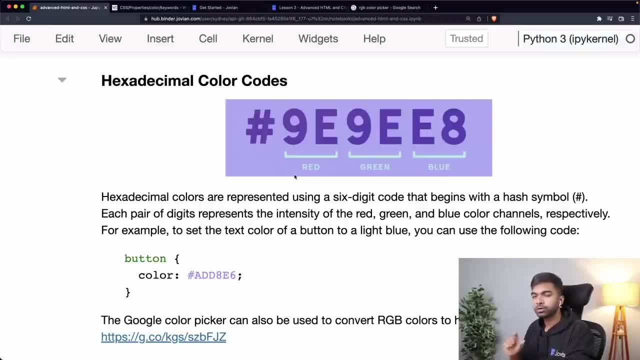 Okay, So this is a representation of RGB, but instead of numbers, you use numbers and characters. Now, this is represented using the hexadecimal number system. I will not get into it here, but the idea here is an hexadecimal color is represented using three, represented using six characters, and each character could have a two, F or zero. 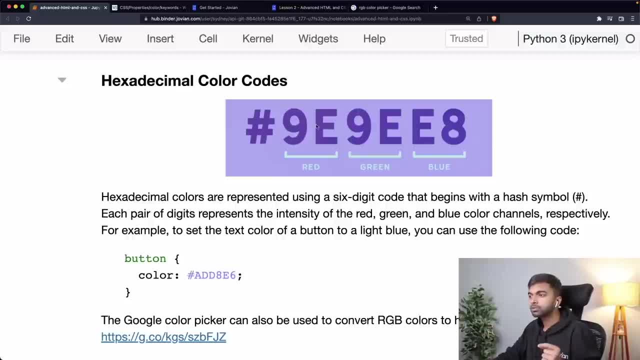 to nine, zero to nine or eight to F, And the first two characters represent red. This is in fact the hexadecimal. Okay, This is the notation for the red value, And then the next two characters represent green and the next two characters represent blue. 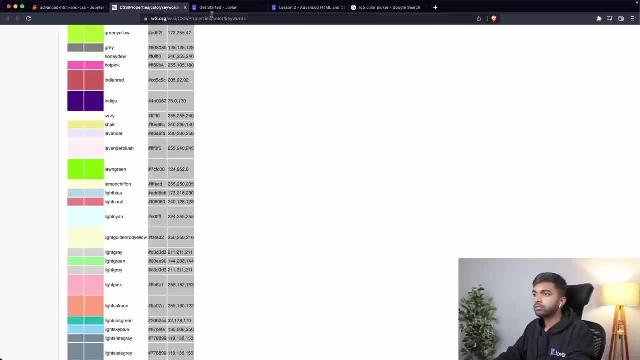 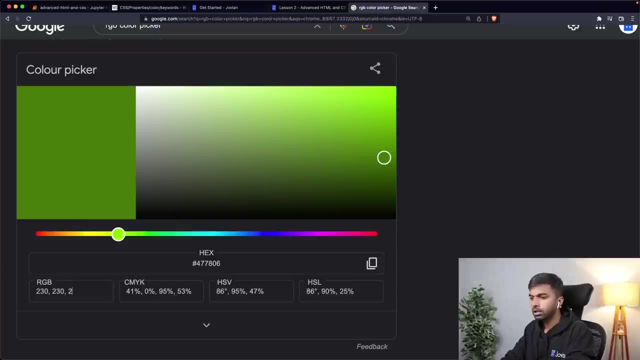 Okay, So often what you can do is you can if you have a RGB color in mind. let's say, the color I want to use in RGB is 230, 230 to 40, I can put that into a color picker and I can get that hexadecimal. 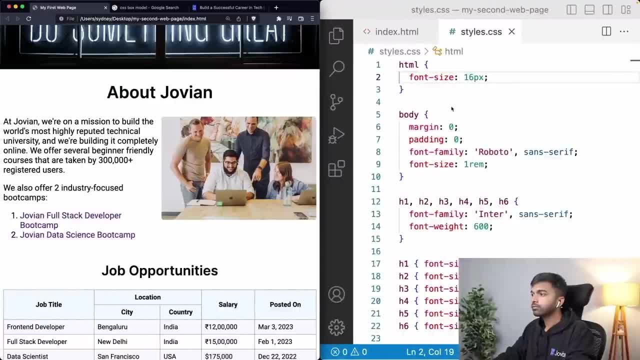 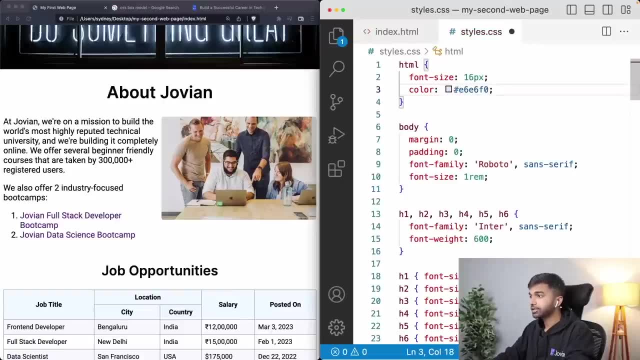 code from the color picker and I can just copy that And instead of typing out the entire RGB, I can just say color is hash. hash includes hexadecimal, and then type out the color here: Okay, And that will just change the color on the page. 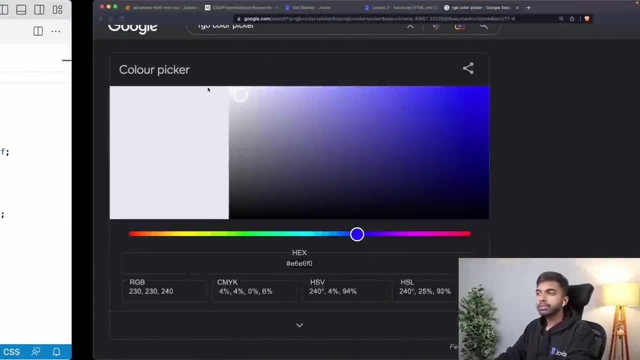 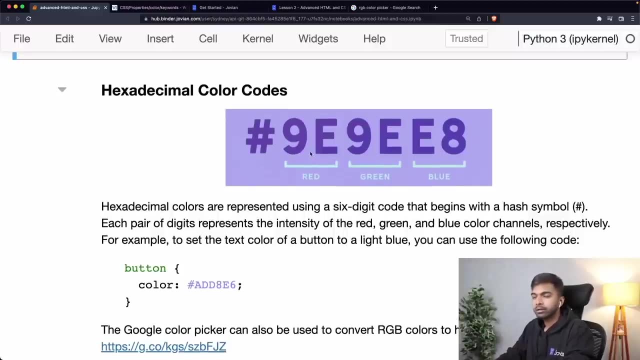 That's a very bad color, but you get the idea. Okay, So RGB and hex are equivalent. It's just that hexadecimal is more commonly used because it's easier to copy paste and use across different platforms. So often you will find colors in hex. 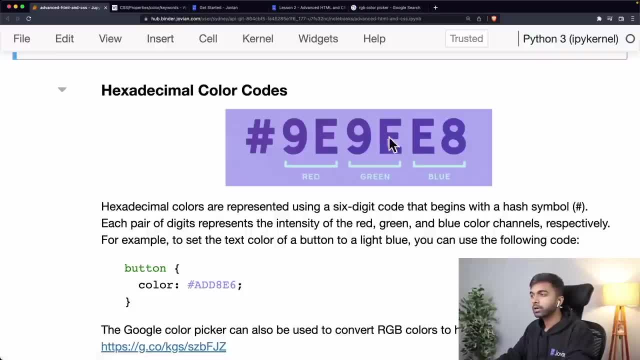 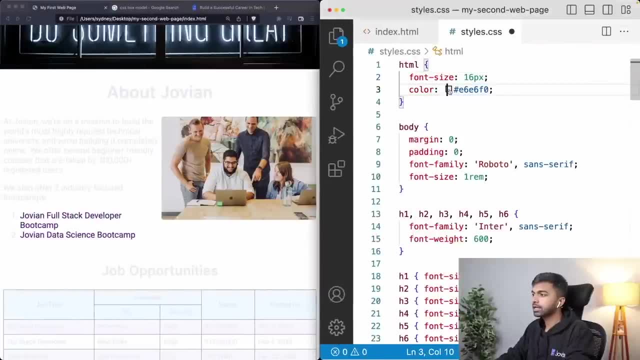 So when somebody says get the hex code or get the color code, This is what they're referring to, And you can always get hex codes online. In fact, a lot of color pickers also give you hex codes instead of RGB. Let's say, I go in here and I go select a very dark color and I click this. 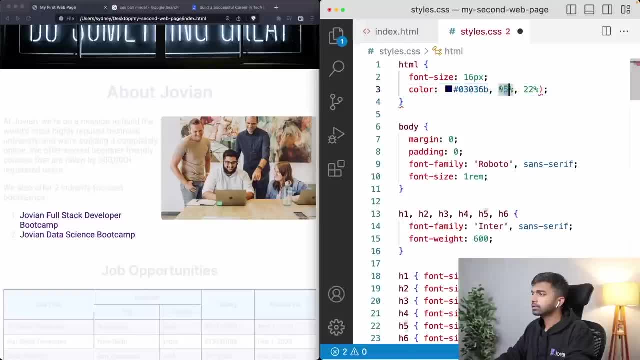 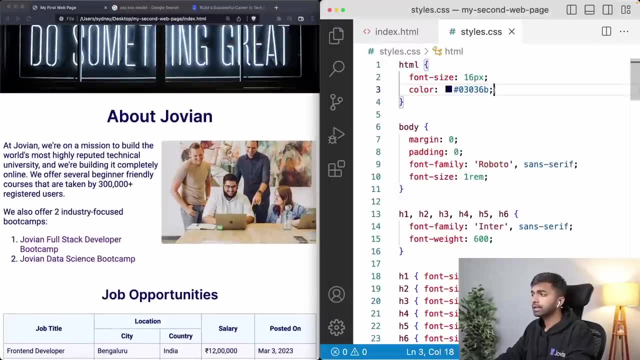 Yeah, I just click that And that is going to get the RGB color for me. Oh, sorry, That's going to get get the hex code off the page for me. Okay, So now I have applied the hex color to it as such. 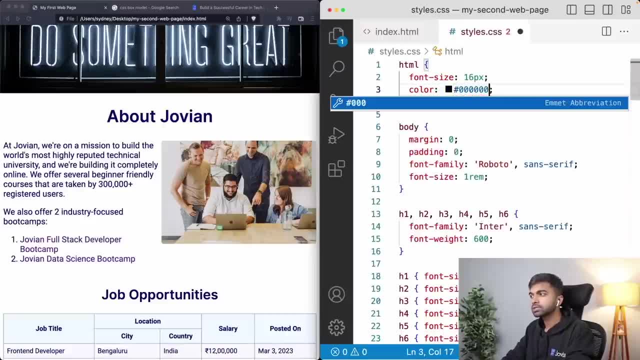 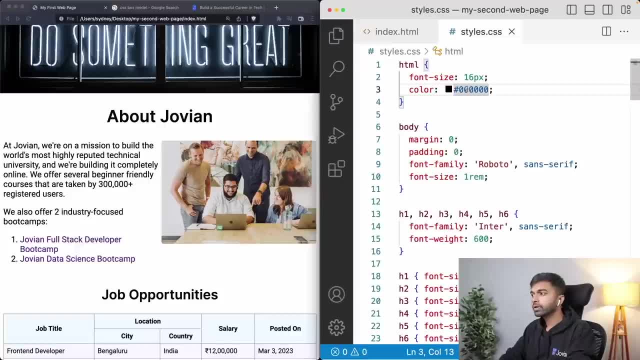 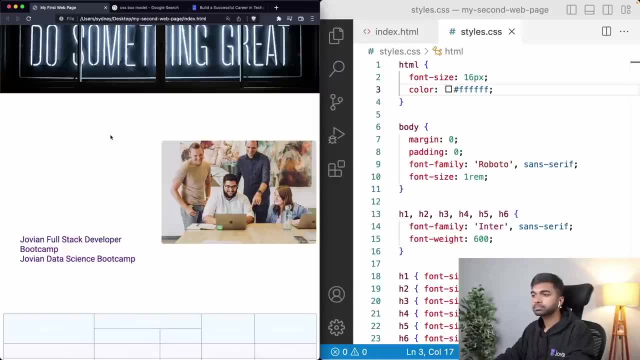 And because each value goes from zero to nine and then eight to F, so F, F, F, F, F, F, that is white. Okay, Now everything has gone white. And of course, if you, if I put zero, zero, zero, zero here, that would be red, and so 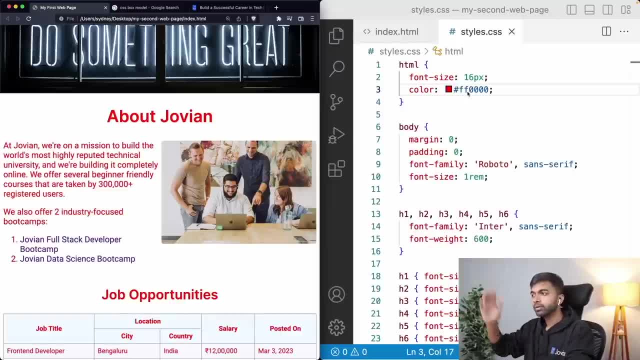 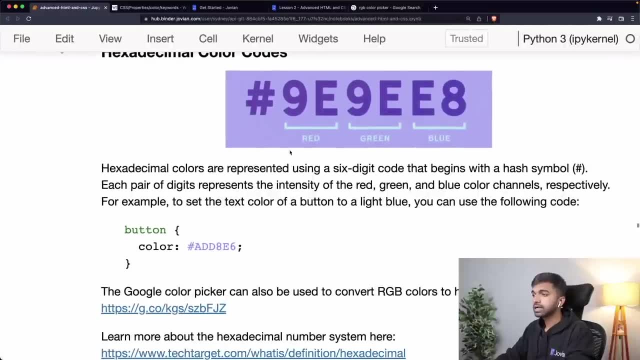 on. So I'm going to put red from zero, zero to F, F, and next two characters are green, Next two characters are blue. Let's get rid of that. So that is the hexadecimal color code, And you can use that to set background colors. 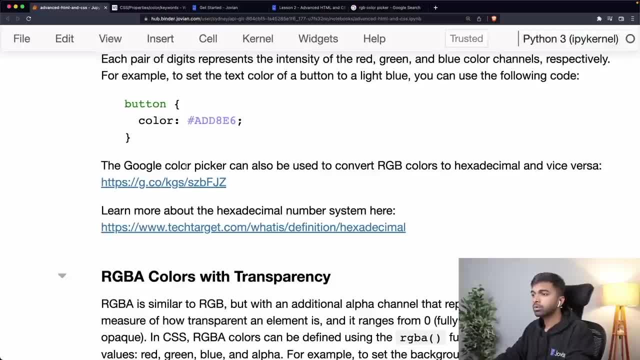 You can use that to select X color. all of that and you can use the Google color picker to convert RGB colors into hexadecimal or vice versa. You can, for example, copy this hexadecimal color code and come into the Google color picker and paste it here. 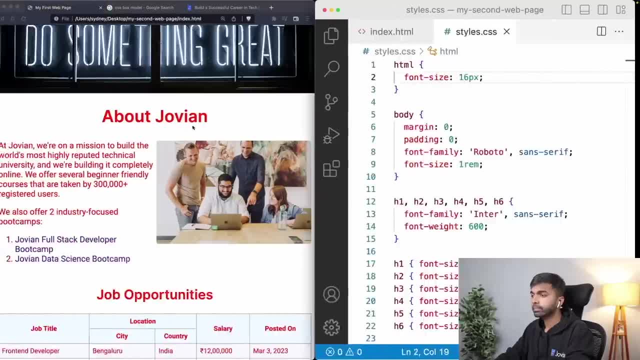 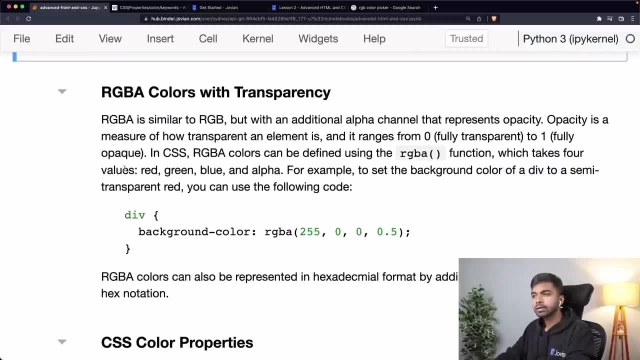 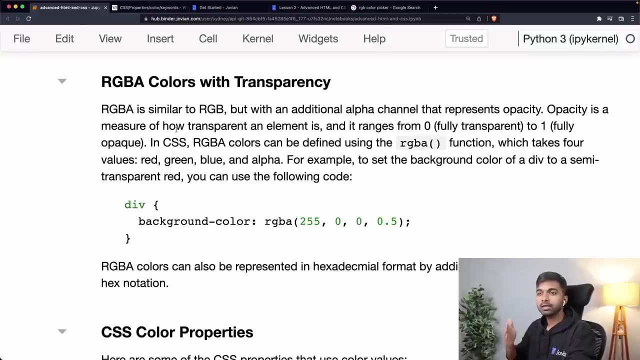 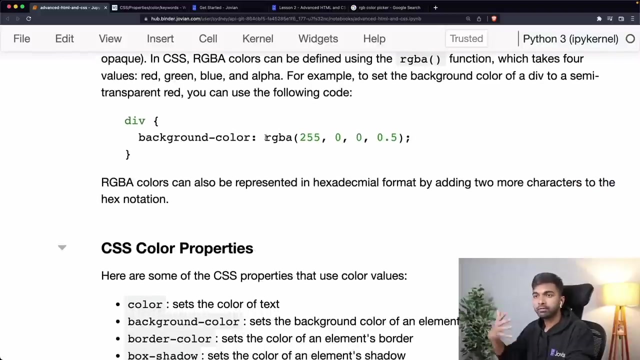 And that will give you the RGB code. Okay, So that's the hex. Another color scheme is something called the RGBA color scheme, which is similar to RGB. You have red, green, blue, but then you also have transparency, So you can, for example, make the background of a div, or you can make the text on on. 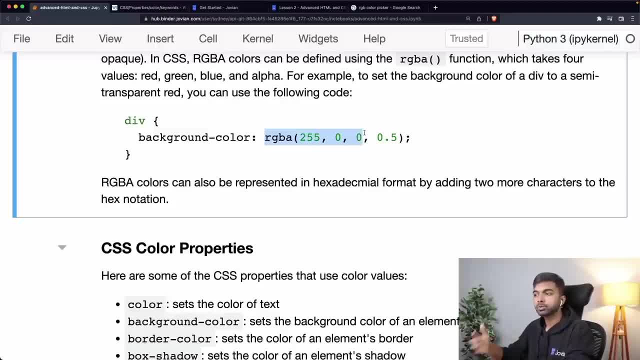 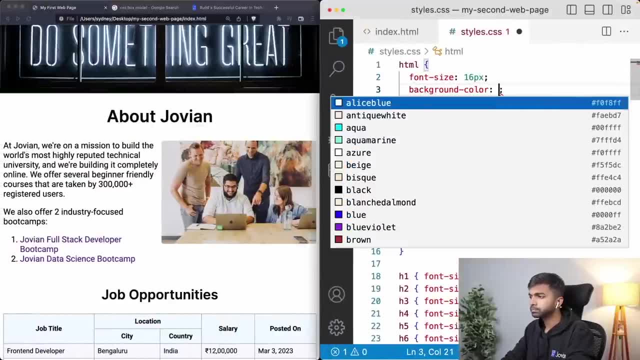 a particular page slightly transparent so that the color behind it shows through. Okay, Let me show you an example. Let us set the background color of the page to, let's say, red. going to look very ugly, but let's set it here. 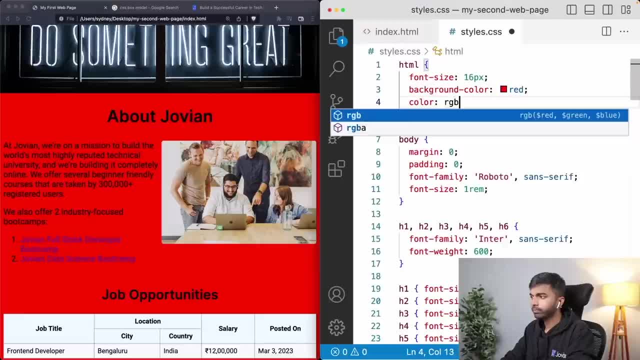 No problem, Then let us set the color of the text to zero, zero, zero, or maybe just 20,, 20,, 20,, which is a very dark green. Okay, It looks very similar. It's still looking Very black, almost close to black. 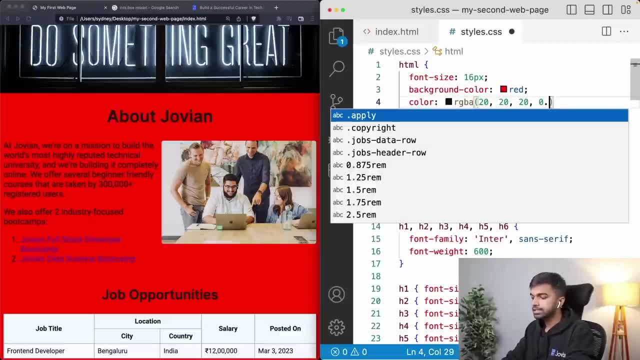 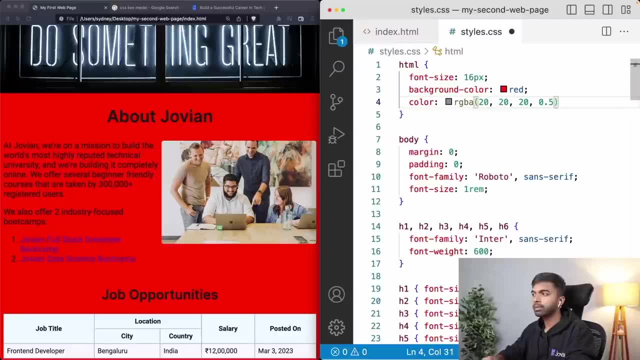 But now let us come in and change this to RGBA and let us set the opacity, or transparency, to 0.5.. So one is, I believe, full opacity and zero is completely transparent. In fact, let's put 0.5 first. 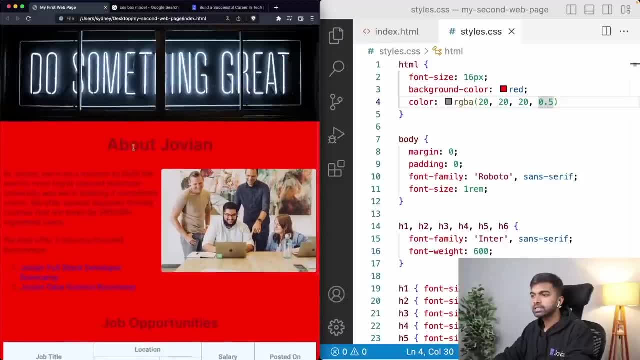 You can see that. you can see some of the red behind. you can see some of the red behind the text. If this were green, you would be able to see some of the green behind the text. Okay, So if I set the transparency to zero or the opacity to zero, now you can't see the text. 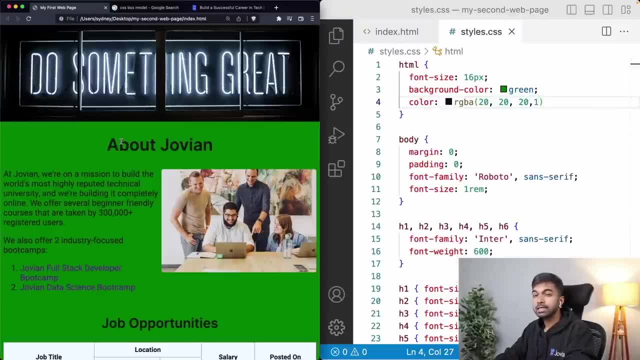 at all. If I set the opacity to one, you can't see any of the background color at all through the text. but somewhere around 0.4,, for instance, you will see that we are able to see some of the background coming through. 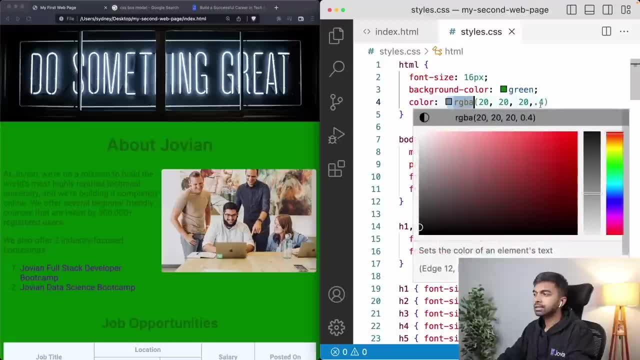 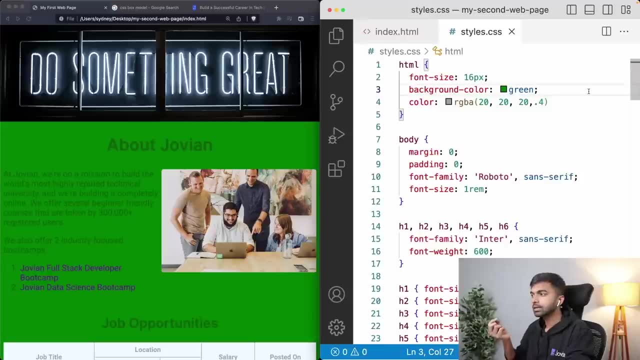 Okay, So you can also use this RGBA and similar to RGBA. there is also the hex code, where you have red, green, blue and then two more characters to represent the opacity, The opacity level as well. Okay, Not very commonly used, but this is also something that you can do. that is about colors in HTML. 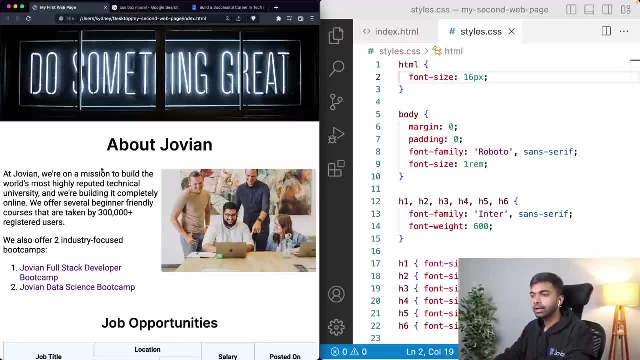 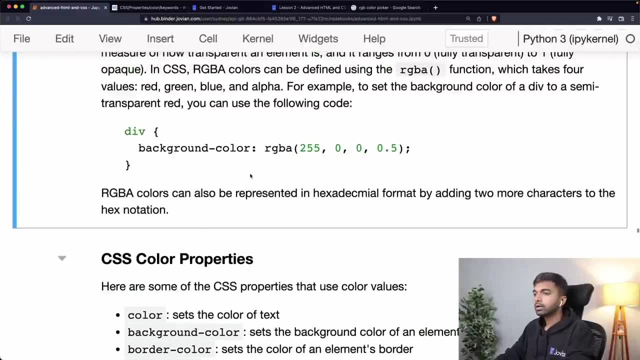 And, as you might've seen, all the color choices that we are making by default look pretty ugly. So we'll talk about how to come up with good colors, but now that you know how to create a color, these are all the different ways in which you can use colors. 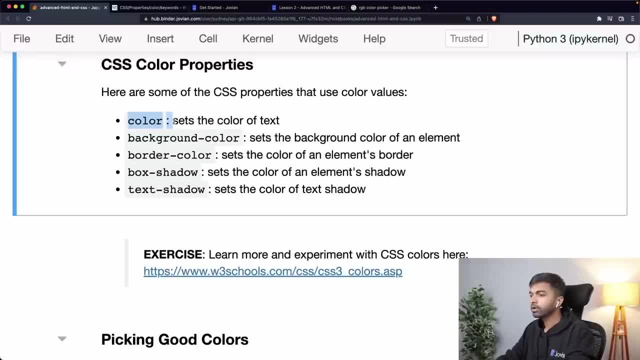 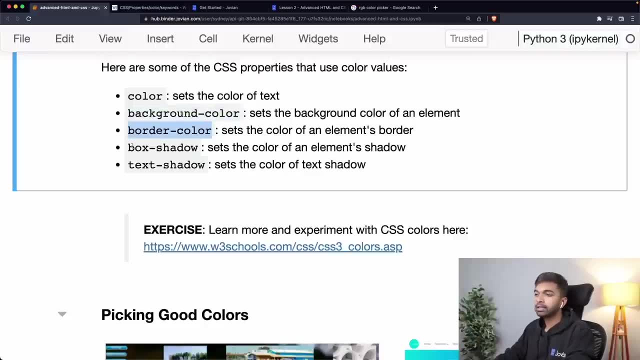 So you can use color to set the color of the text, which is what we've been doing right now. You can use background color to set the background color of an element. We've done that as well. You can set the border color and then you can use box shadow and text shadow. 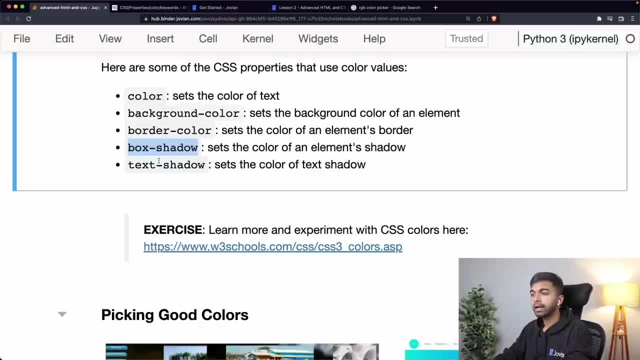 So box shadow is used to create a shadow around a box or a div, and text shadow is used to add shadow for text. Okay, So you can look up the properties specifically and see how these are set, but I'll just show you an example of border color. 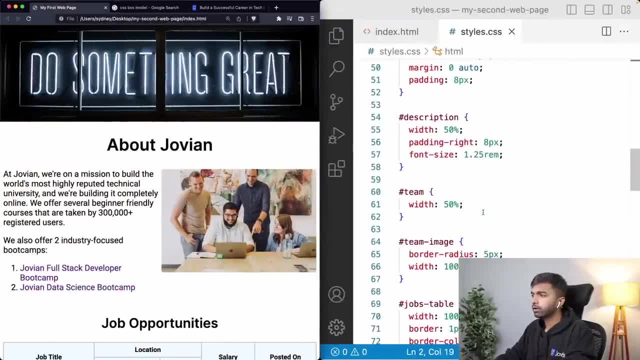 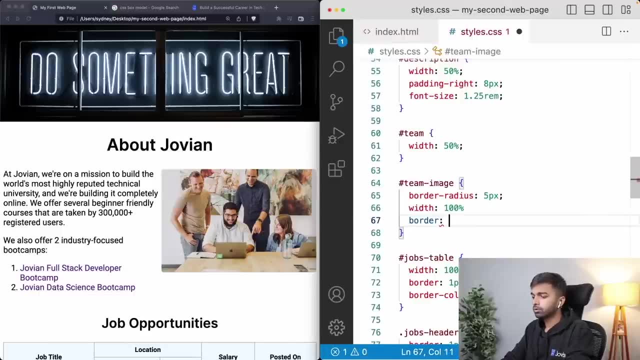 Let's say we can come here and we can set for the team image. We can set The border width, or we can just set the border to five pixels solid And let's pick a color: deep blue or something like that- Dark blue. 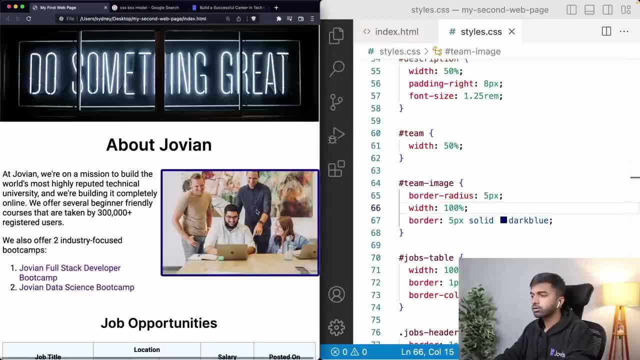 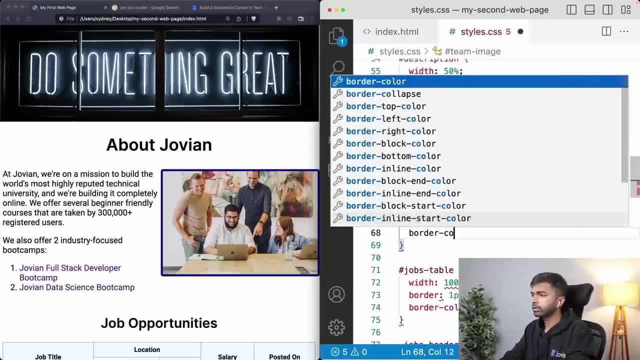 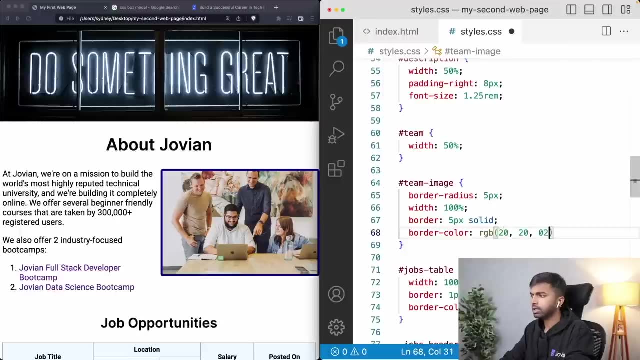 Yeah, Now you can see that there is this dark blue border and I can, in fact, just change the border color separately. So I can say border color: Okay, RGB, and let's say 20,, 20,, 20, and that gives it a blackish or a dark gray border. 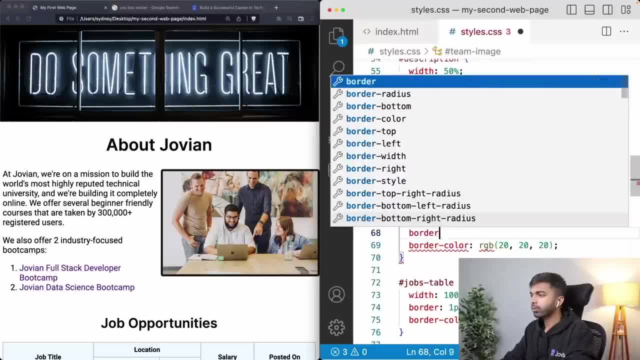 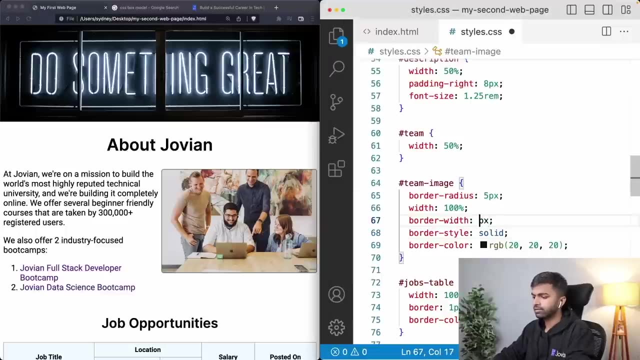 And I can also set these border properties separately. So I can set border width to one PX and get rid of this, And I can say: border as solid is a solid border. Well, let's make that five PX, This is a solid border. 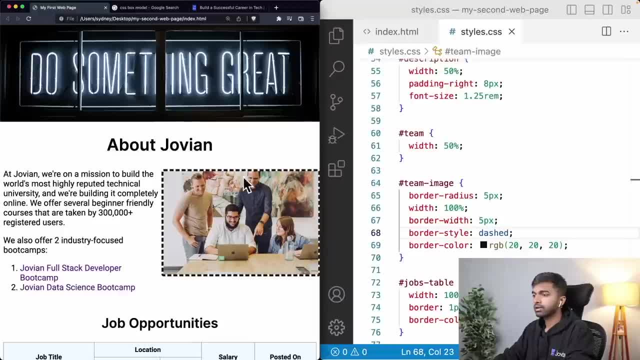 I can also have a dashed border. You can see that we can have a dashed border like this- not very common but you can do it if you want- And you can also set maybe the width of different borders So you can say border left to it is five pixels, that you have this border only on the left. 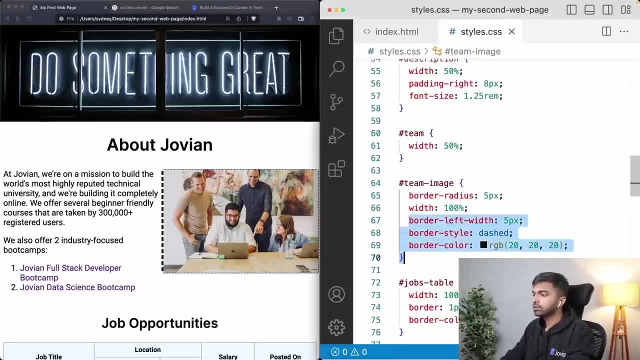 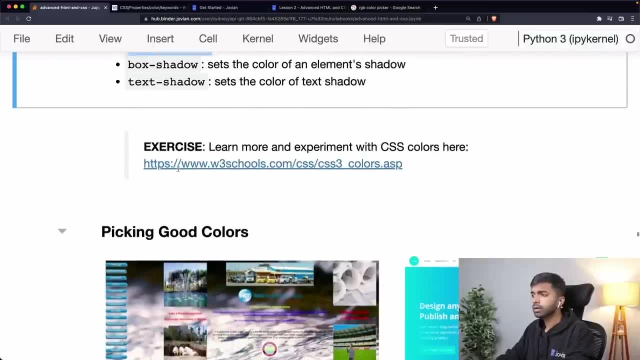 and everywhere else You just have a one pixel border. Okay, We have all these ways in which you can specify borders, and you can specify the styles of borders and colors of borders as well. So again, except for this. So again, experiment with colors a little bit. 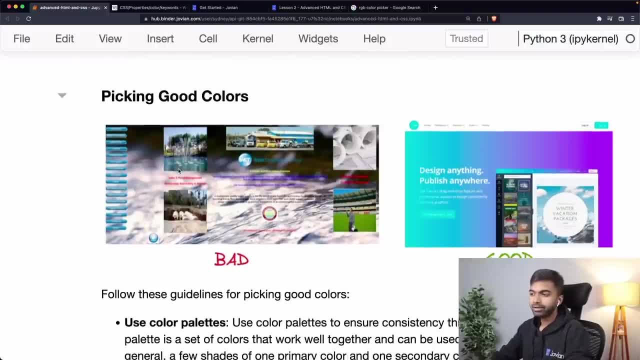 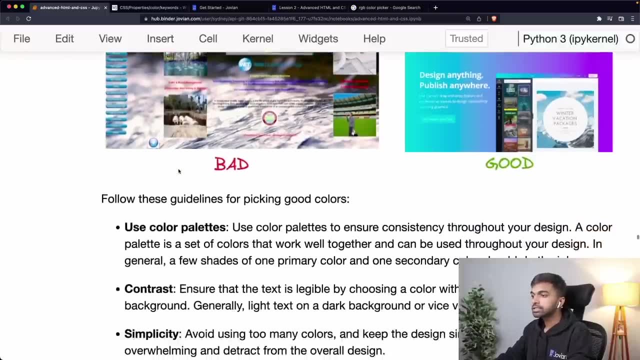 And, generally speaking, picking good colors is really hard, And if you're picking at random or just looking at some colors and trying to use it, that is you're going to have a tough time. So here are some guidelines for picking good colors. 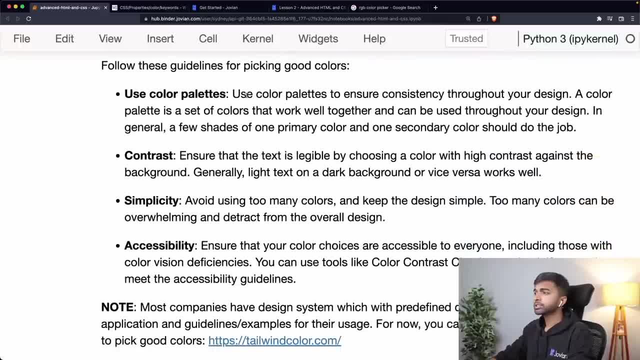 The first is to use a color palette. to use color palette to ensure consistency throughout your design, and a color palette is a set of colors that go well together. So color palette will typically have a primary color and some shades of the primary color. 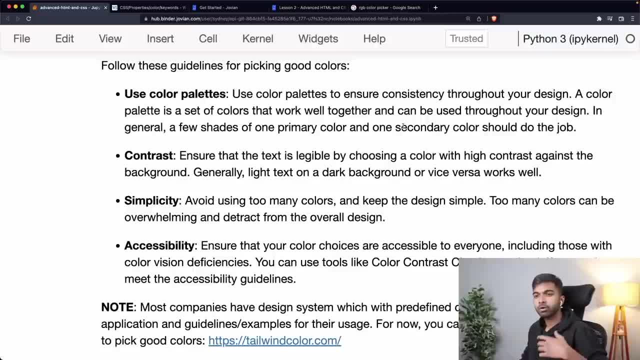 Which are often used either for text or for, maybe, buttons or for backgrounds. Then you will have a secondary color which is also used sometimes for buttons. You may not have a secondary color at all And then, finally, you should have a, maybe a few shades of gray that you're going to. 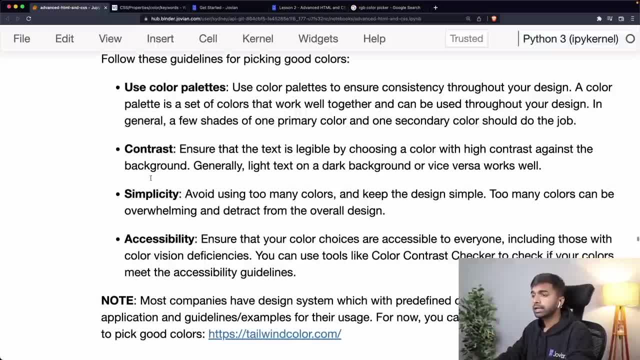 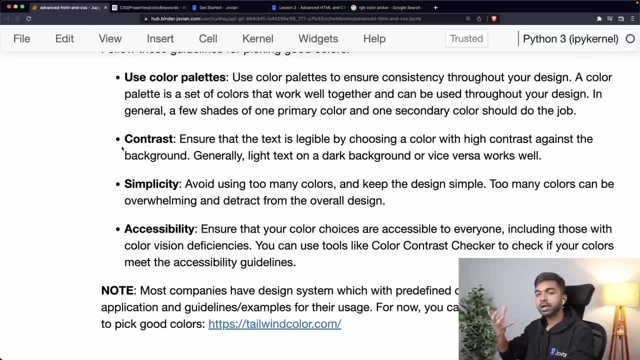 use as backgrounds or as text colors. Then one other thing to keep in mind is contrast. You want to make sure that the text is legible, which means that the text should have- should have- a high contrast compared to the background. Okay, 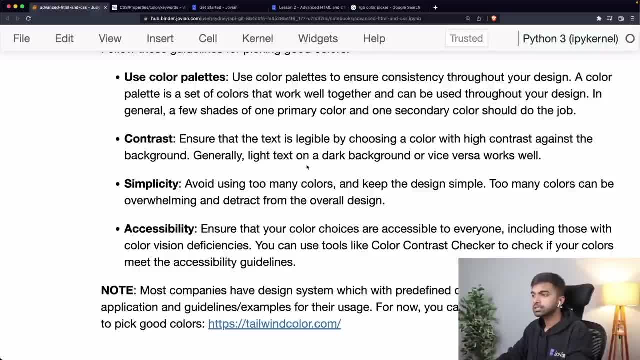 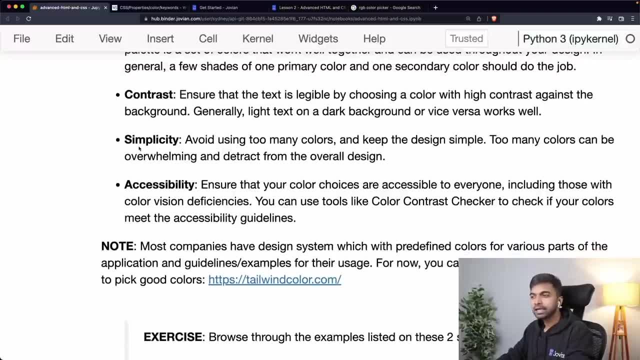 If, generally speaking, you're not able to read the text, Then that's a bad color choice. So light text on dark background or dark text on light background works well Then. the other thing is simplicity: avoid using too many colors just because there. 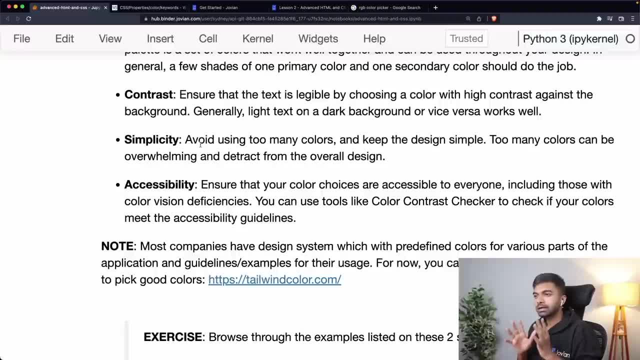 are all these colors doesn't mean you have to use them. Just use, as I said, a color palette with a primary color a few shades and a secondary color a few shades. even there stick to one or two shades. All the texts on your page should more or less have the same color, and ideally should. 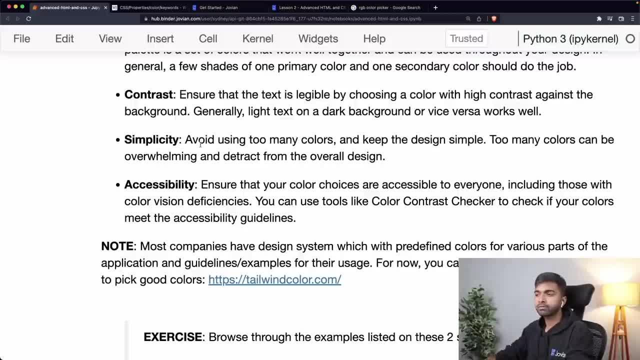 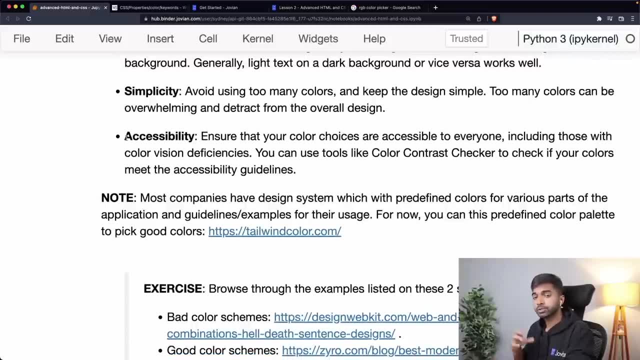 just be shades of gray, maybe with a slight tinge of blue or slight tinge of green, depending on the theme of your website, And finally know that sometimes there are issues like some people have color blindness, Some people do not have a perfect vision. 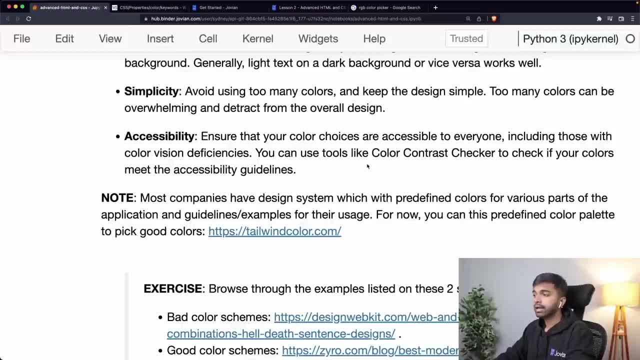 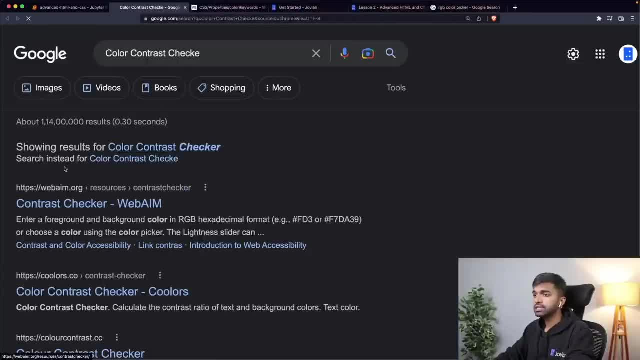 So there might be color vision deficiencies that your users might have, And then you can use tools like color contrast checkers. You can just search online for color contrast checker and you can paste some HTML code here. or you can like set the foreground color, background color and you can check what the 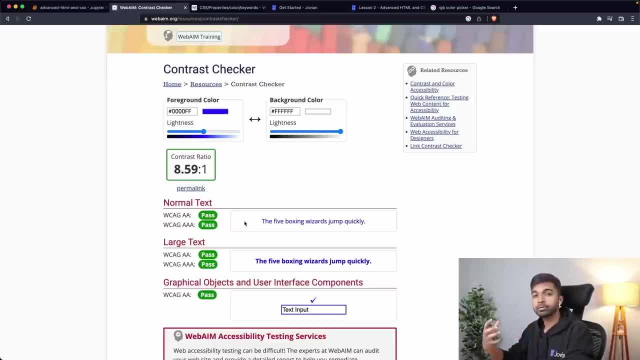 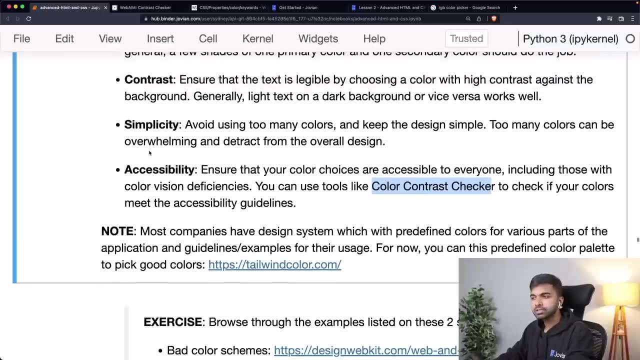 contrast ratio is, And it will tell you whether this is going to be Readable for somebody who has color vision issues or general reading issues. All right, We'll just keep those things in mind Now. generally, most companies have a design system with predefined sets of colors for 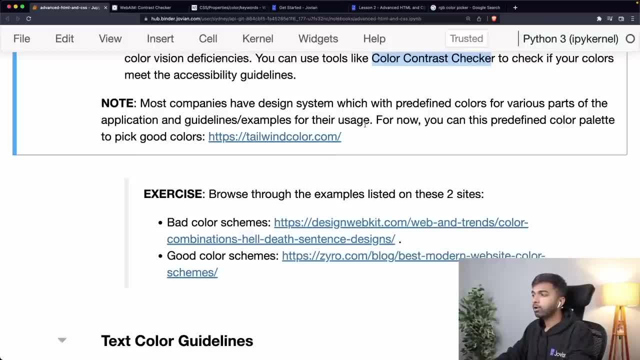 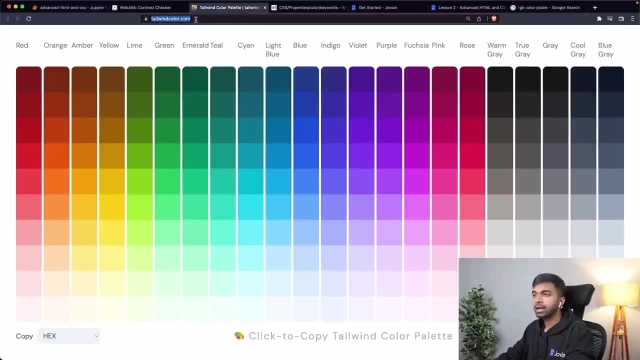 various parts of the application And for now, you can just use this one color palette. So what I would suggest is use this color palette- tailwindcolorcom- It's linked in the notebook page- And from this color palette, For whatever website you're working on, pick a primary color. 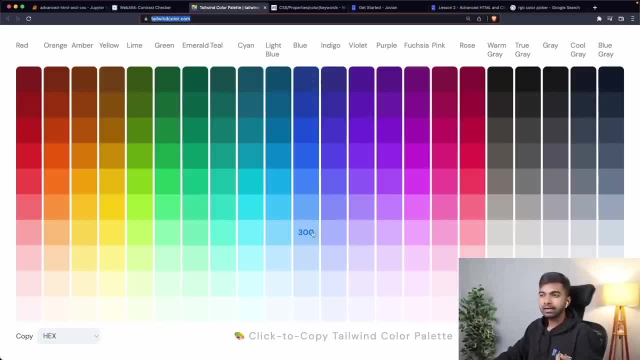 In my case, I tend to almost always go with the blue and pick a secondary colors. The primary color is what is going to be used in most places, And then the secondary color is going to be used in some other places where you need a. 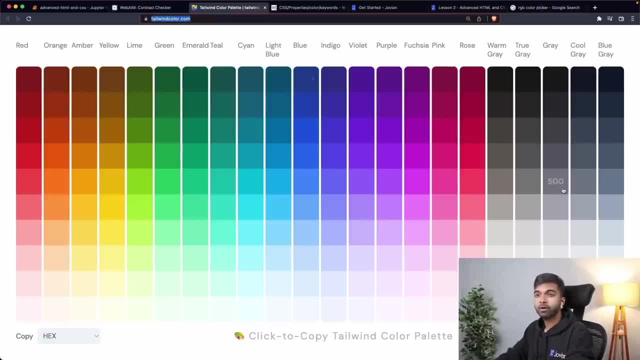 second color And then maybe just use the different grays for showing text. Okay, So that is what I would suggest: Pick a primary color, pick a secondary color and pick a bunch of grays. Don't use the predefined CSS colors. 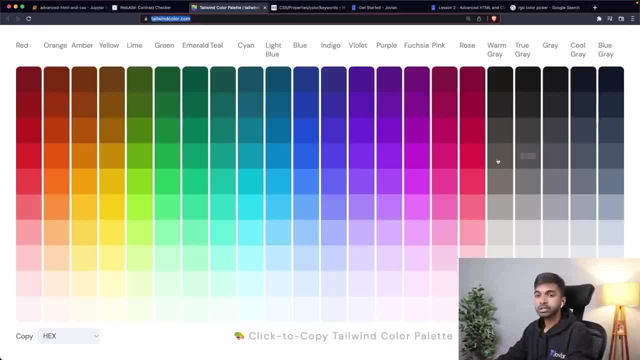 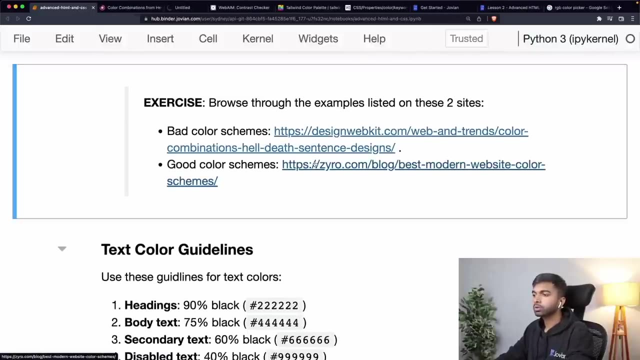 They don't go well together. Don't use random choices of colors that you find, come up with or try, or you're trying to figure out using the RGB color picker. that generally doesn't work. Use a color scheme. Okay So, based on the color, based on these, I would also encourage you to go through some example. 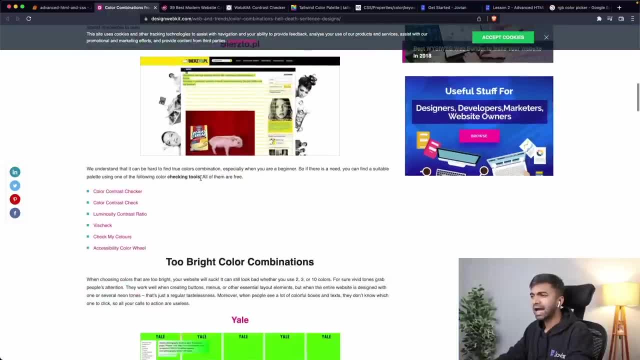 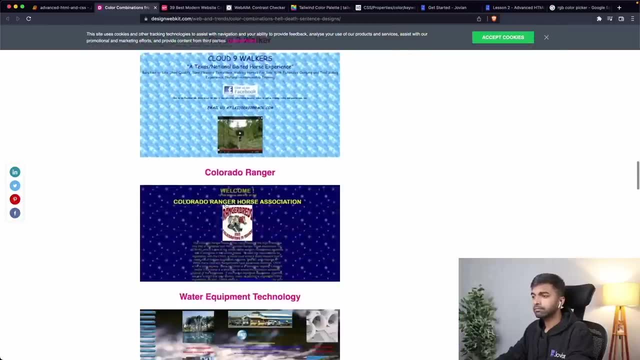 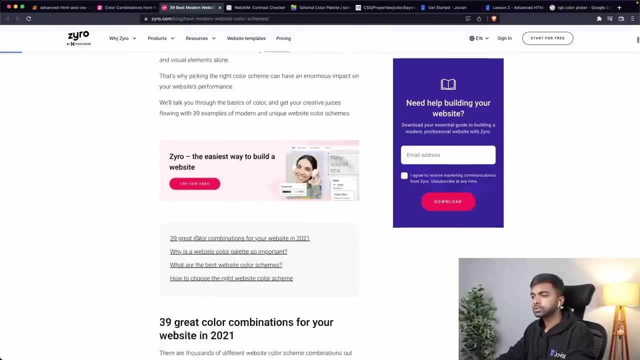 sites here. These are some examples of bad color choices. I mean this was not too bad, but it's still too bright. I would say these are all all completely fairly bad color choices. This is, You see, a lot of that, a lot of this earlier in the internet era, and these are some choices. 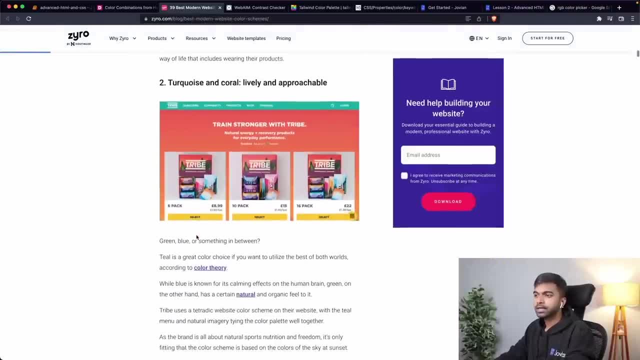 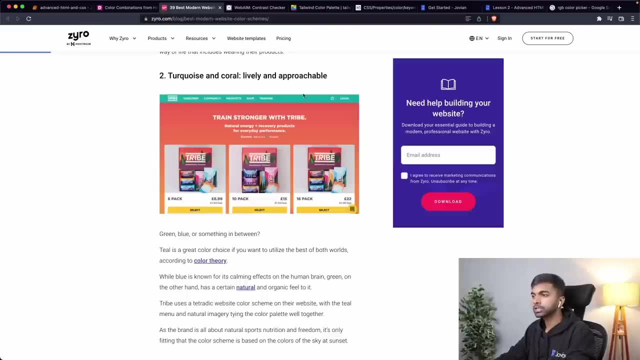 of good colors. So one thing you can do for your website is just pick color combinations. You can see that there's a primary color which seems to be orange, and orange and yellow, So some shades of orange and yellow. in the secondary color here seems to be this blue. 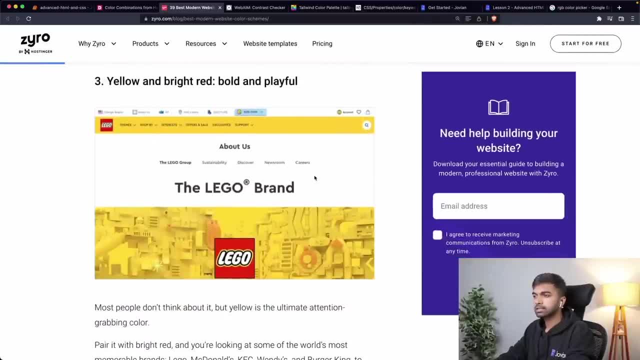 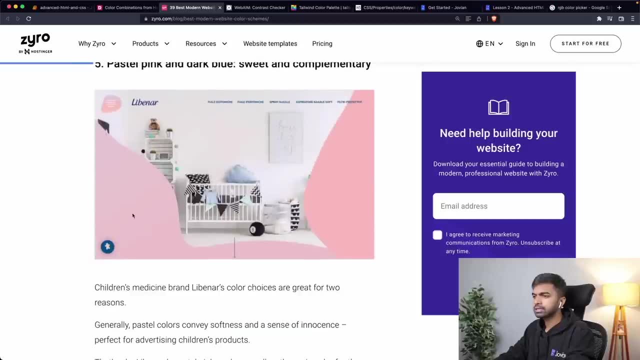 And here again there is this primary color of yellow for Lego, And there's there's no second. there's a bluish secondary color that is used in some places. here The blue is a primary color, And here there's the same. there's this: I don't know what this color is called, but 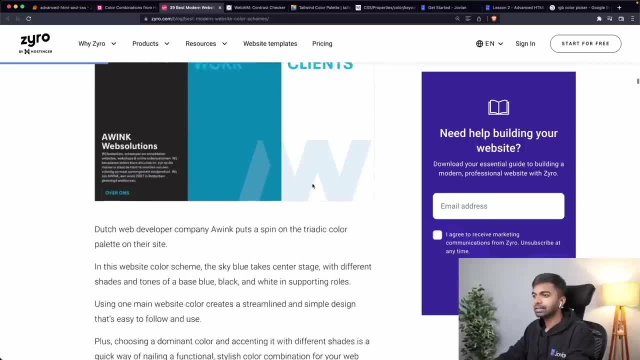 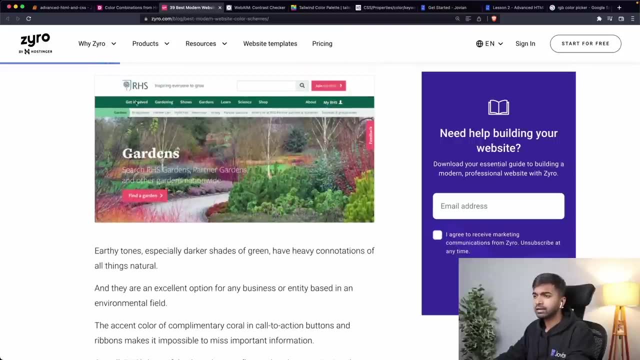 this like light pink color, probably again there's this primary color, secondary and then maybe like a black secondary color. Sometimes you can use images and matching colors with images, So you have the green color, shades of green, and then you have a secondary color which. 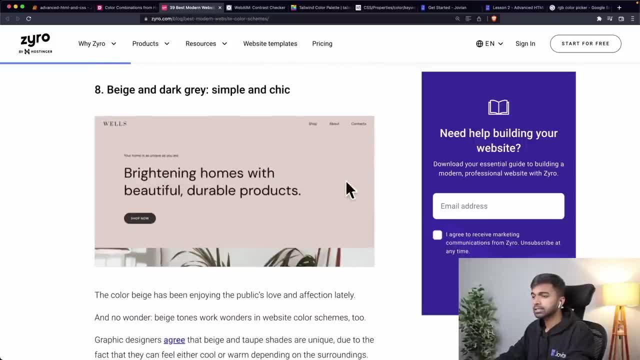 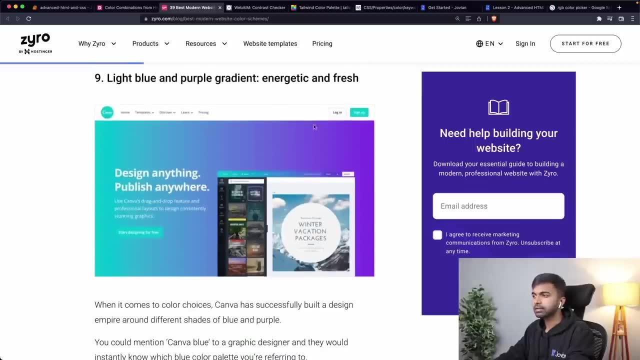 is the red, That's great. A primary color, this color, and then the secondary is just black. here Again, here we have this gradient which is basically just shades of the primary color, And then the secondary color also just seems to be a shade, or maybe these are the two. 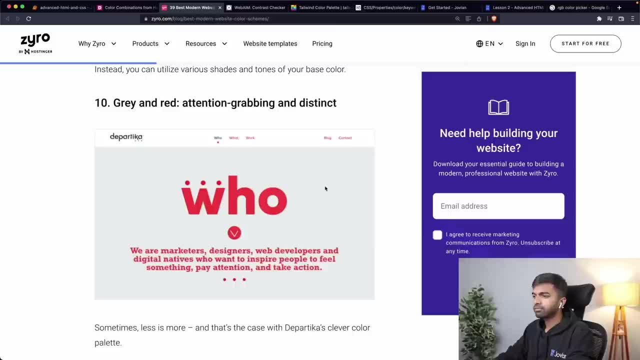 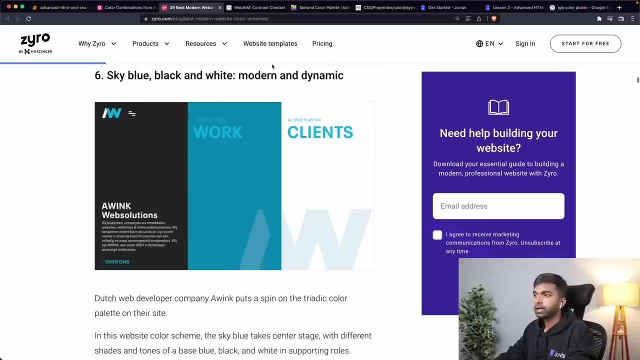 colors, primary and secondary, And again, here we have gray and we have red. So yeah, look at examples, look at your favorite sites and just copy what they do and use a color palette of tailwindcolorcom while you're designing your website. 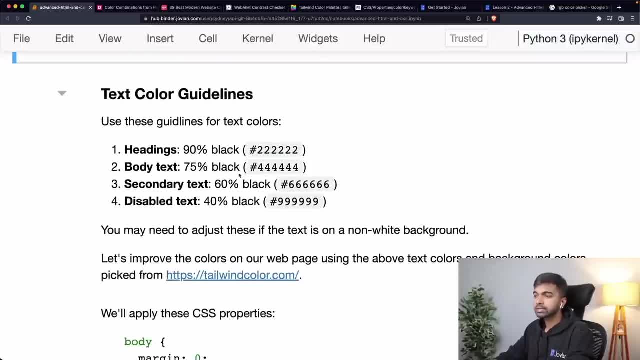 Okay, Specifically for text, I want to share a few guidelines. Normally, text should be almost always some shade of gray, some shade of black. Okay, You can have a slight tinge of blue, or a slight tinge of green or red, depending on your themes. 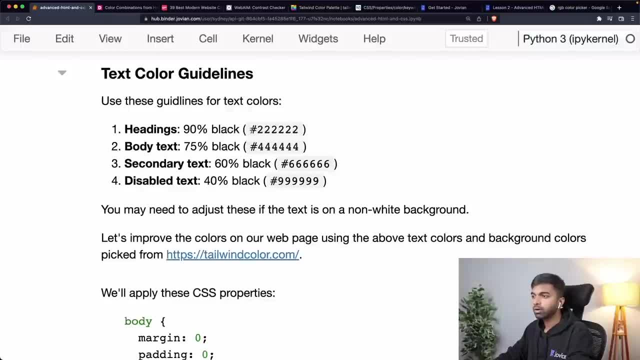 But here's a good guideline. Your headings can be 90% black or just 2,, 2,, 2,, 2, 2, 2 would be the color hex color. Your body text can be 75% black, or 4,, 4,, 4,, 4, and any secondary text. that is not important. 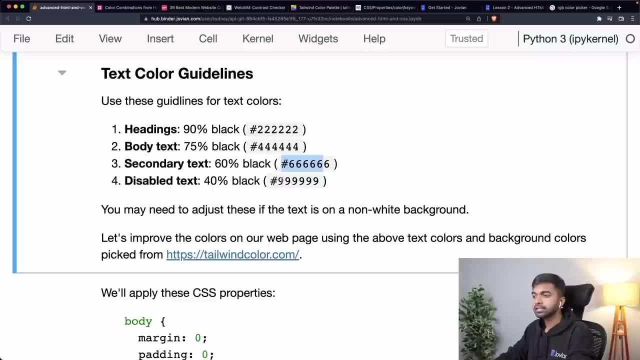 can be 60% black, which is 6, 6,, 6, 6, and disabled text should be 40% black. So it's a bit confusing because black is zero. the 90% black is going to be very close to. 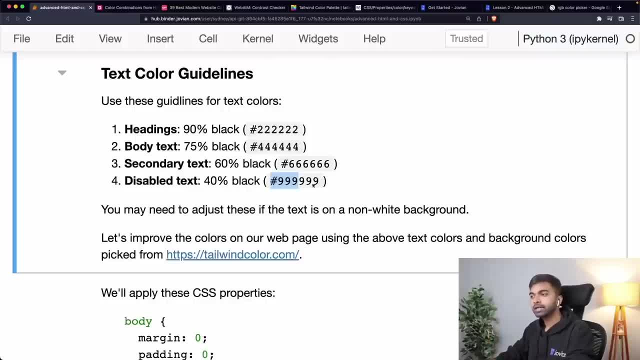 zero and 40% black or 60% white is going to be very close to FFF, right, But I hope you get the idea. Hex colors can be a bit confusing to wrap your head around, but as you practice more you'll get used to it. 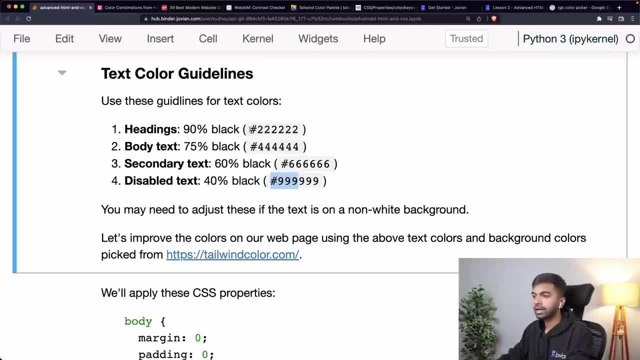 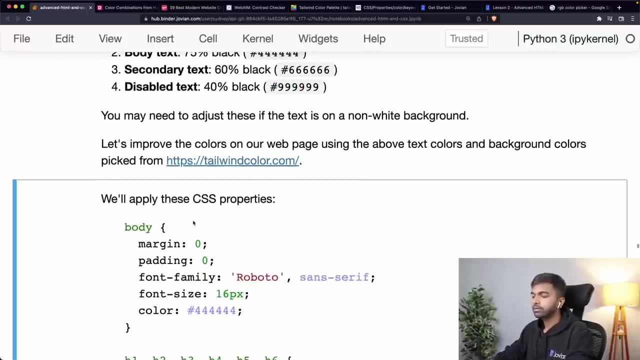 Okay, Closer to zero is dark. away from zero is white, is light. but 90% black is very close to zero. Let's do that. Let's come in and let's set these colors. Let us first come in into our body and let us set. 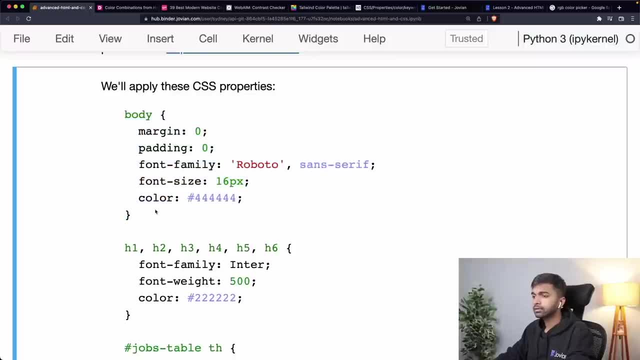 These. Okay, Let's set the font size and the color to the color We're going to set, to 4, 4,, 4, 4, or 75% black. So let's come in here to the body. 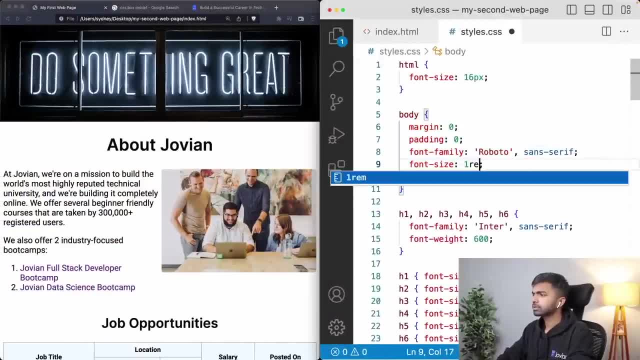 We've already set the font size to one REM. I think that should work. We have just added the 4,, 4, 4, 4 color and our body text is slightly gray, but it still looks fine. but I think the headings can be made slightly darker. 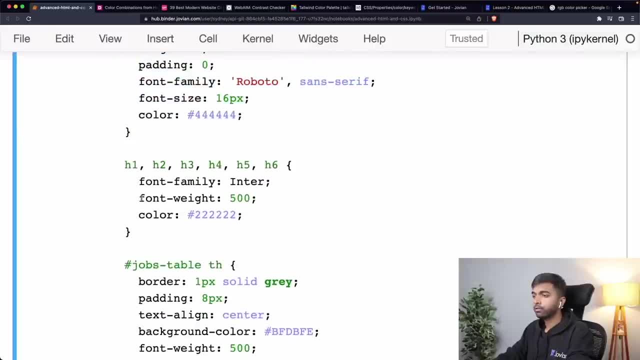 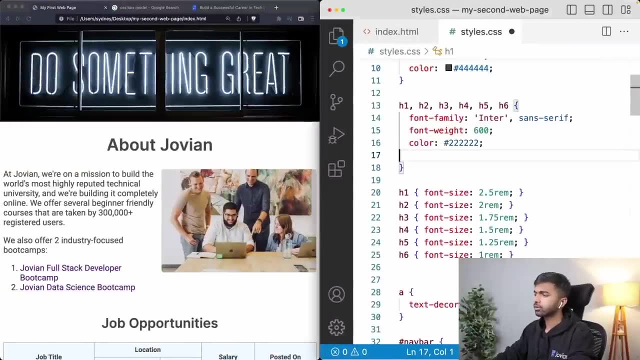 So let's come into the headings, and for each of the headings let us set the font weight to 500 and font color to 2,, 2,, 2.. So I think I'm going with 600 here. I like 600 looking good for me. 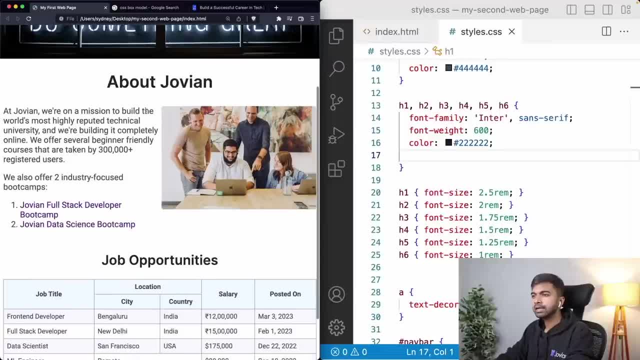 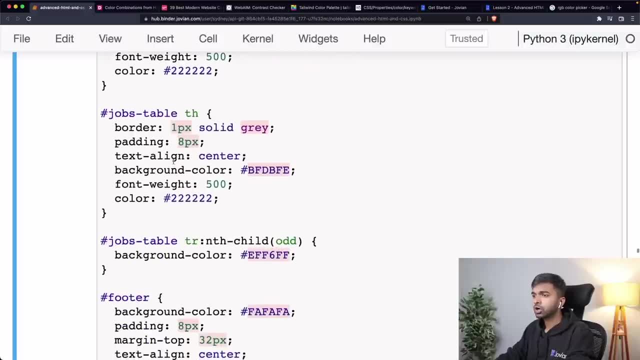 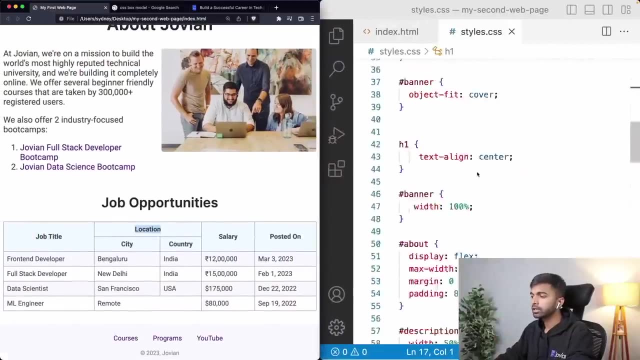 So I'm just going to set the color to 2,, 2,, and now our headings are slightly darker. So that's fine. Then what else? Well, we have this jobs table. on this job table, I want to make these titles slightly darker, because they are more important, more prominent. 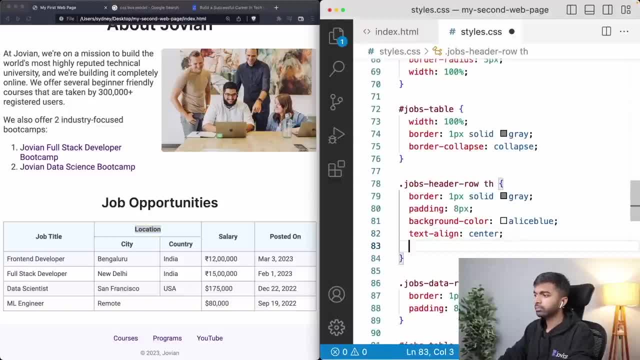 So I'm just going to come in into the jobs table and into the row header I'm going to add the color Oh 2,, 2,, 2,, 2, 2,, which is the same color I'm using for the headers. 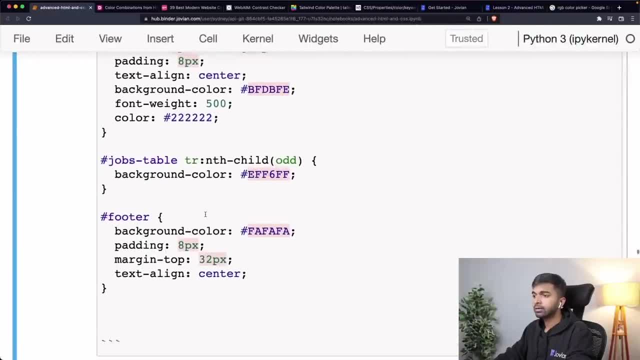 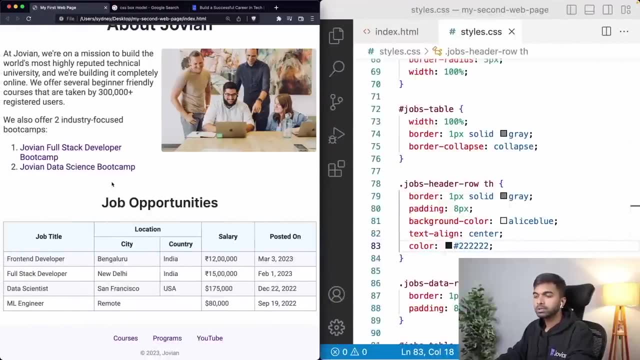 Now these are a little darker, so that's great Then. okay, Now these backgrounds, right? So remember, I said we don't want to use the name colors, we want to pick from a team. So generally for for backgrounds of tables, you can use maybe the primary color and a. 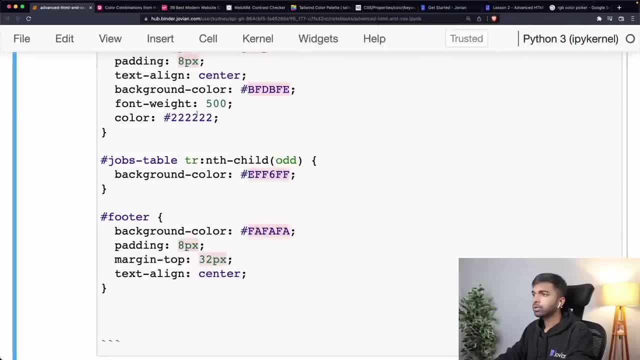 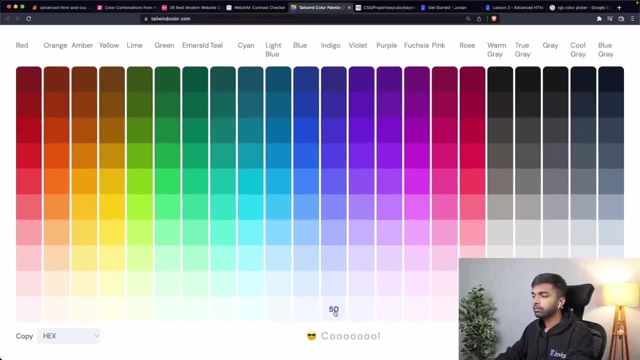 very light version of the primary color. So let's see, I'm going to go in here into tailwind color palette and I'm going to pick the lightest. I'm going to pick a version of Indigo or my row background. 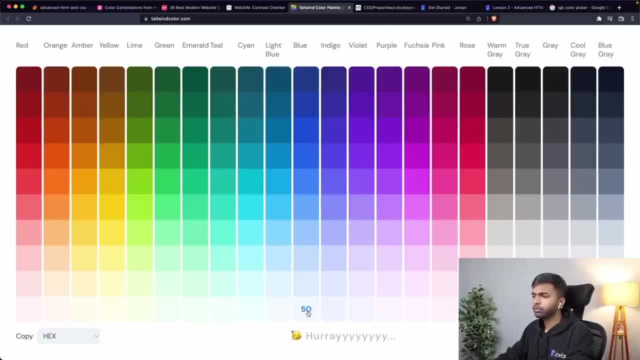 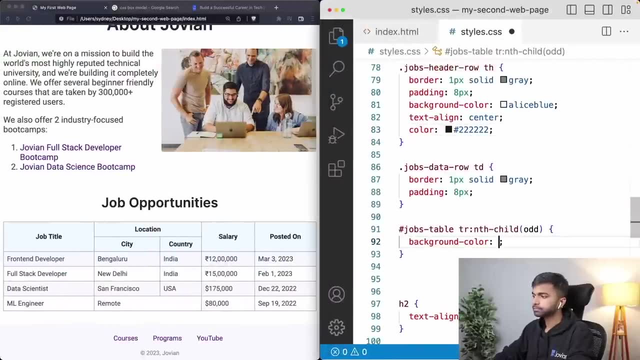 So it is simply Indigo 50, or let me, let me pick blue 50, just to be very safe. And when I click on it it copies the hex code, So I can come in here into the nth child and I can paste this color. 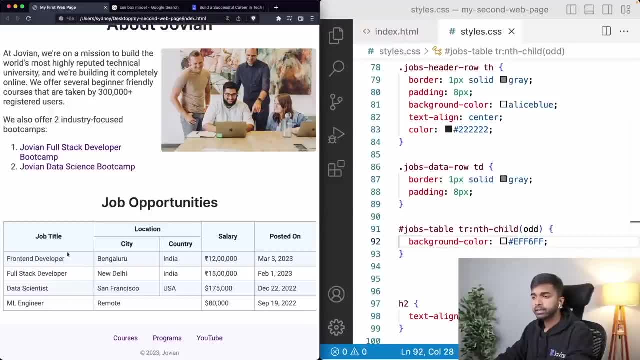 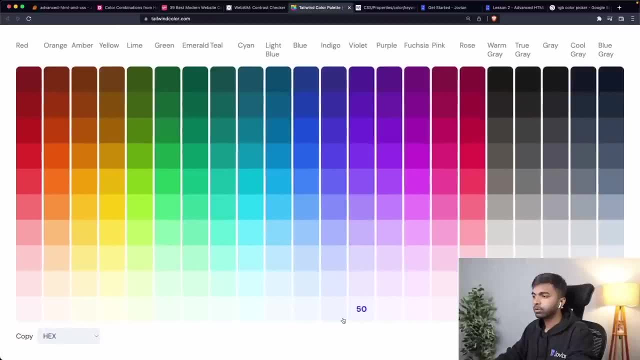 And now I have this very light blue that is behind the uh, behind some of the rows, as a background color, And for this let me pick maybe blue hundred, or I could also pick The secondary color, but for now let me just stick with brew hundred. 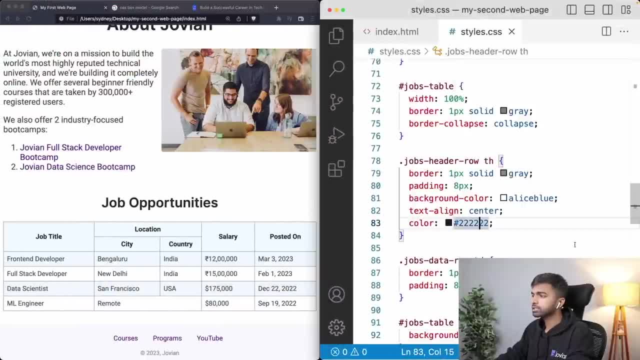 And I'm going to set this on the header row. I'm going to select the background color not as Alice blue, but as this darker, slightly darker blue, So you can see now that it looks slightly nicer, because these two are shades of the. 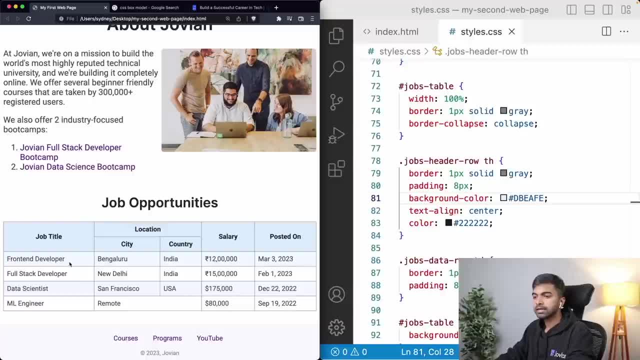 same color, essentially. So this is a slightly darker blue, This is a slightly lighter blue. I could also maybe experiment with blue 200, if I am not happy with the contrast. but that's the most I would go. I would just go up and down within the same um, within the same shade. 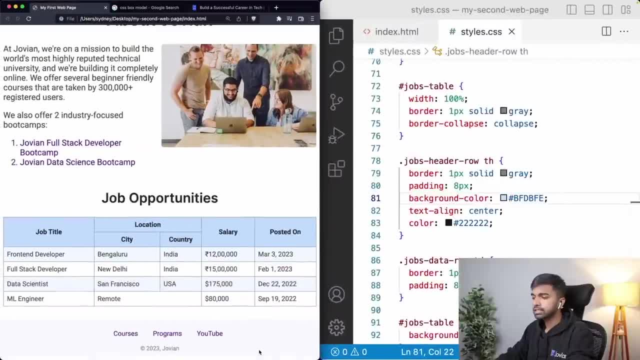 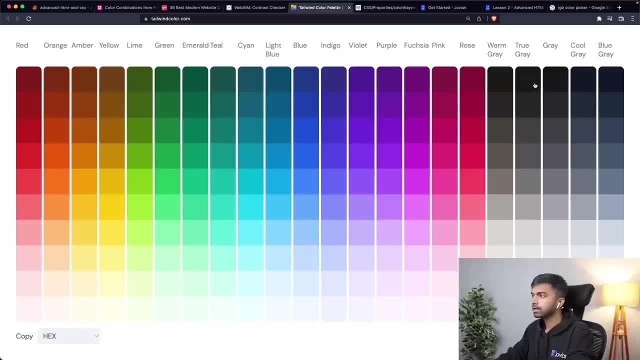 And maybe let me come in here and let us also set the background for this. So you have this footer here generally for footer backgrounds or for body backgrounds. you just want to use gray and you just want to use the lightest of grays. 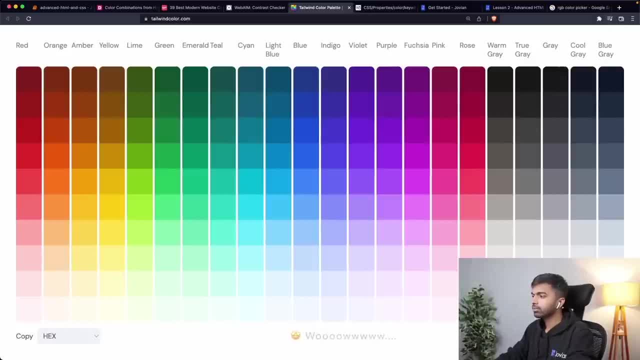 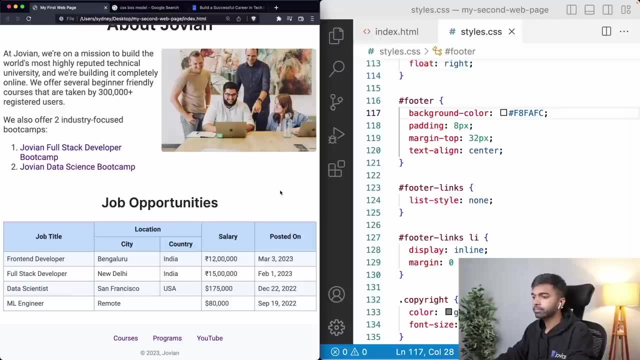 So I have a blue gray here which is slightly bluish gray. So let me just copy the blue gray and let me come into footer and set the background. instead of ghost white, Let me set it to blue gray, And now that looks slightly nicer. or I could even just have used a simple gray as it is. 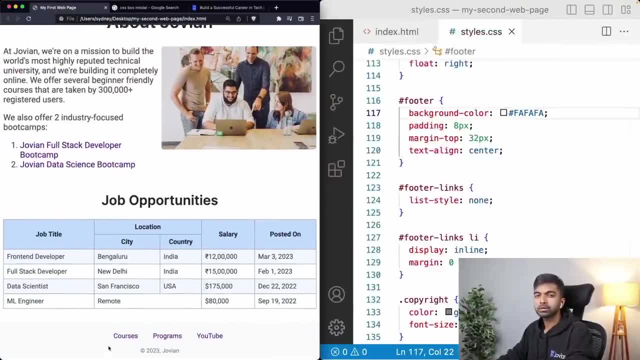 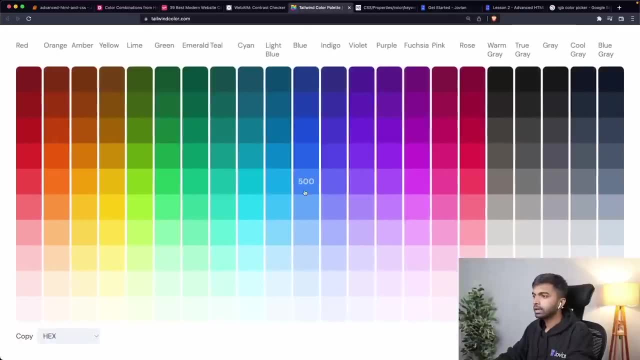 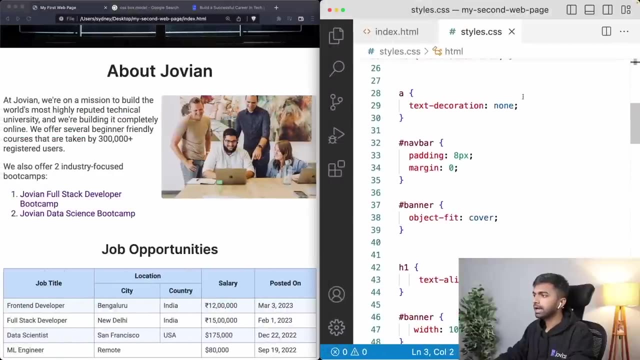 Okay, FAA, and that looks fine. Finally, for the links on this page, I might want to use the blue color so I can just go in and I can pick if um the 500 blue or links on the page. So let me pick the a tag and let me say color 500. 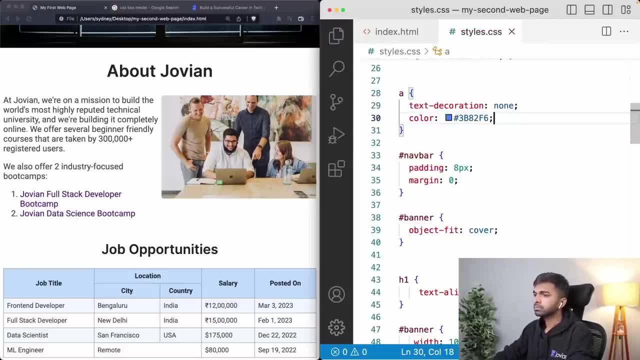 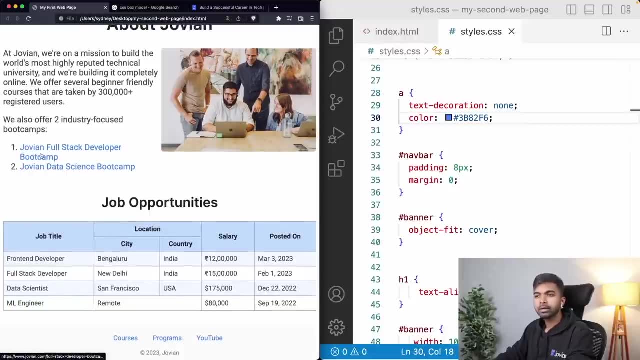 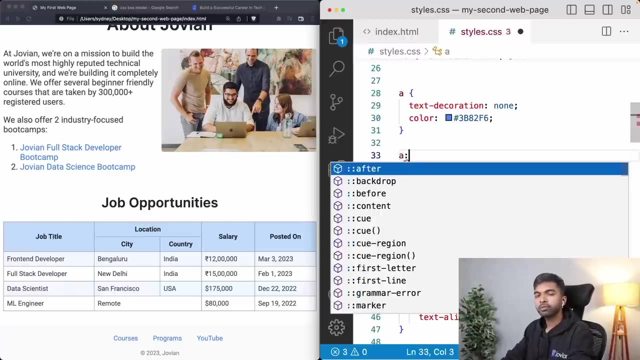 Oh, sorry, Okay, That color. the links on the page will show up like this, but now you can see that, as I hover over a particular link, the color doesn't change. So this is where you can actually use something called a pseudo class or a hover state. 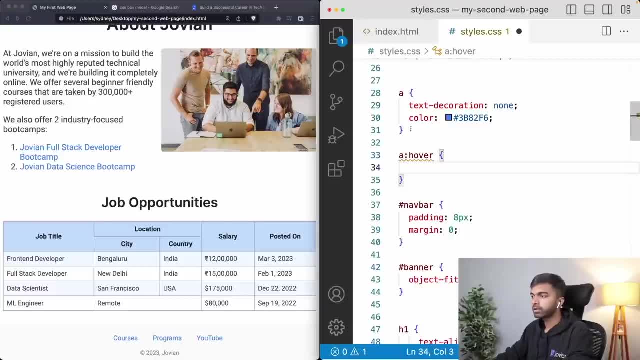 If you want to change how a link looks on hovering, they can say colon hover And now you can put in a different color. Let me make it 700. So let us check. set the color to 700 over here for the hover state. 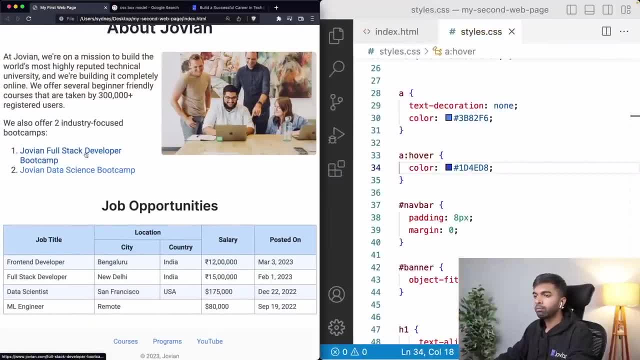 Okay, So now when I hover over a link, I get a different color. Okay, And there are various hover states- We'll talk about them in a future lesson- or various pseudo classes that you can apply, But basically, whenever you're styling links, you should specify your normal color and you. 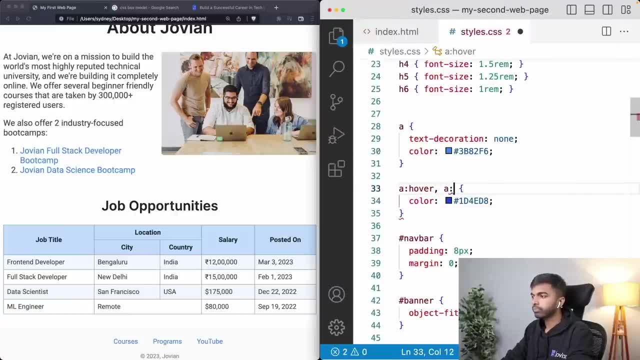 should specify a hover color, And sometimes this hover color- um over- is used when you use the mouse, but when you tap using the keyboard, um you can use, I think you can use focus or active or something like that. So when you are using the keyboard, then the focus color gets applied. 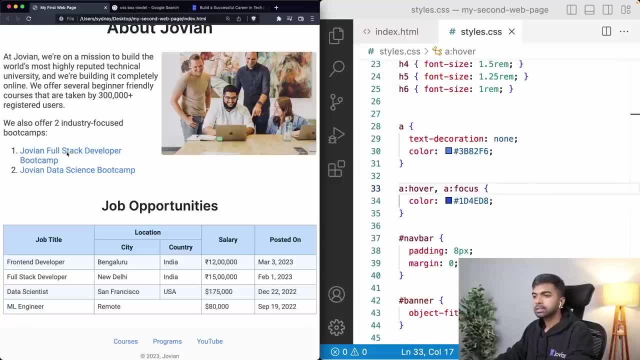 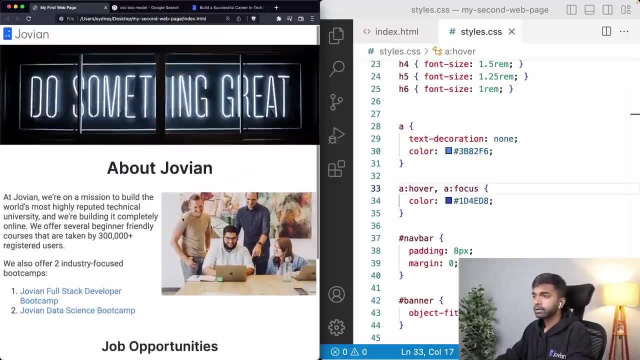 So both hover and focus should generally be set together. Okay, So that is about setting colors. So now our page is looking rather nice because I'm using a consistent color scheme. That's good. What else? Well, we have a gray here. 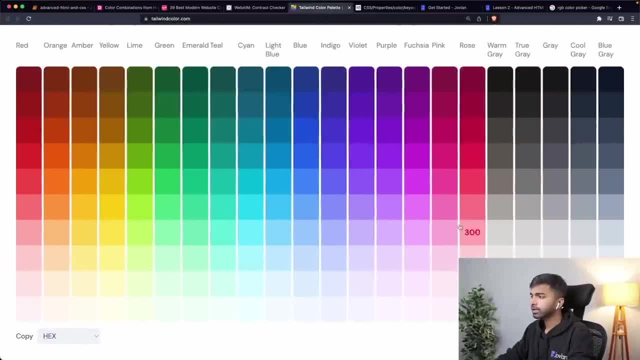 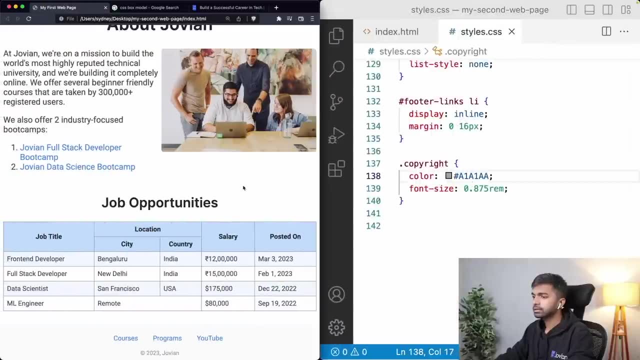 So the gray for the copyright, I'm again going to just grab one of the grays from: yeah, maybe gray 400 or gray 400 should be good enough, And let me just paste that. Okay, I think I was. yeah, that's great. 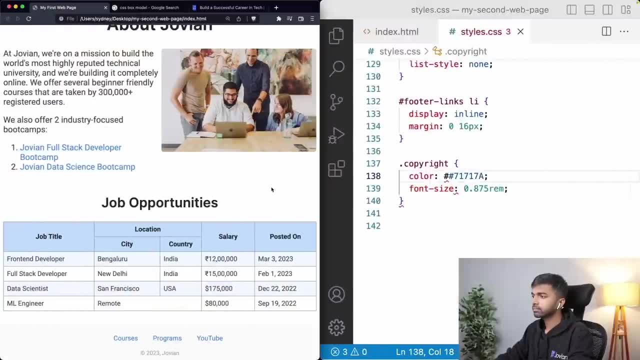 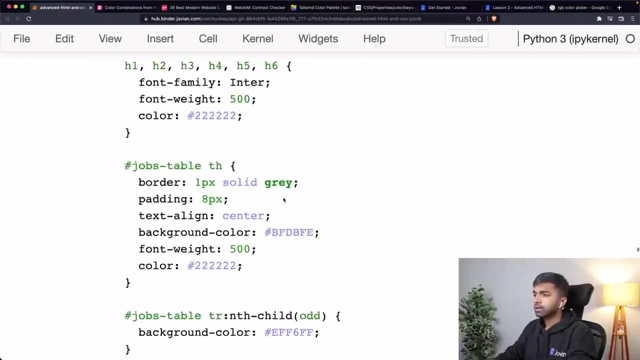 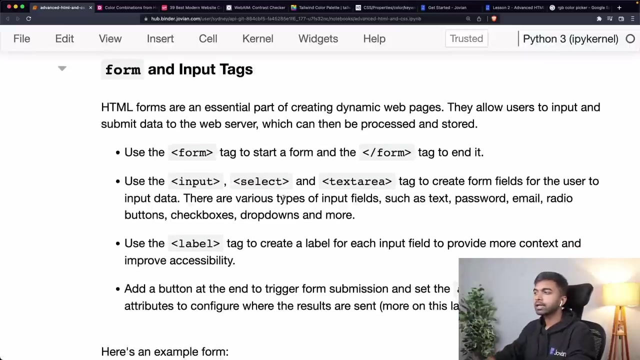 500.. I think I'm happy with that. Okay, So our page is looking nice. We have picked a nice set of colors, So let's continue now, And let us talk about forms in HTML. Now, HTML forms are an essential part of creating dynamic web pages, because they allow users 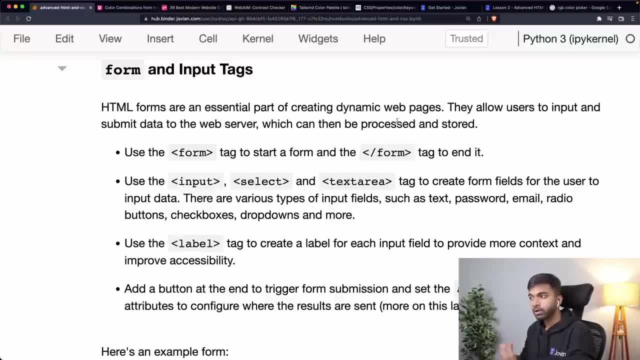 to input and submit data To a web server, which can then be processed and stored. In fact, most web applications that you'll see on the internet are built using forms, and forms are going to become increasingly important as we go further into the course. 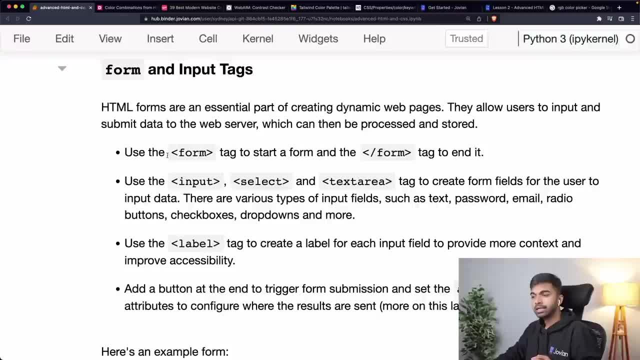 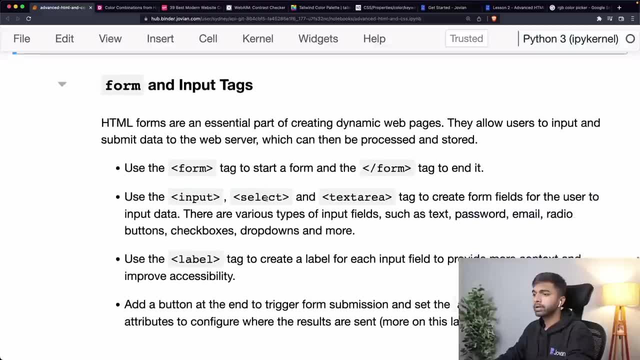 and in the program Now the form is created. a form in HTML is a. no doubt you've used several forms, So you know what forms are. this is what they look like. You can put in some information. forms are created using the form tag. 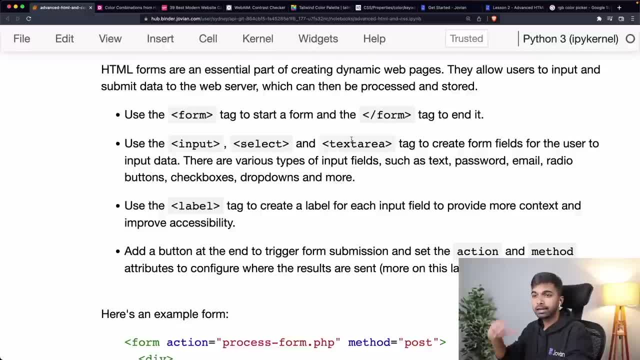 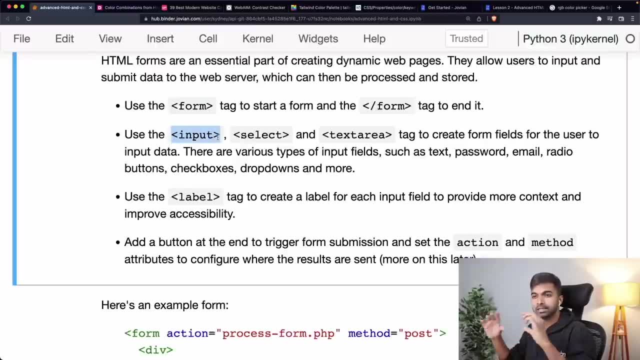 So you start a form tag and then you put a form tag at the end And you put the entire inputs, et cetera, inside it. You can then use three types of tags. You can use the input tag to create these text boxes or other various types of inputs. 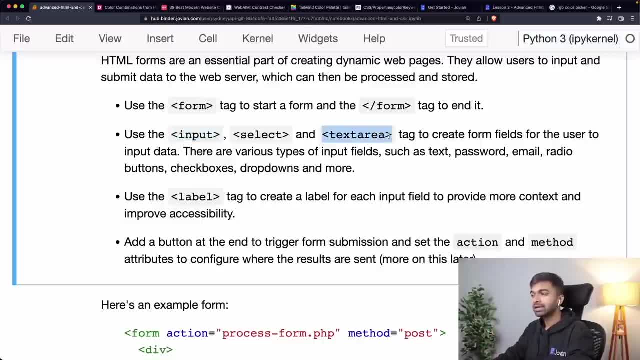 You can use a select tag to create dropdowns. You can use the text area tag to create big text boxes where people can enter full paragraphs of text, And there are various types of input fields like text. You can have password input fields, which is what you do when you log into a website. 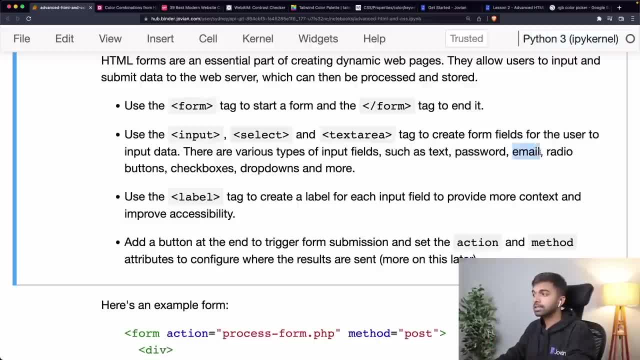 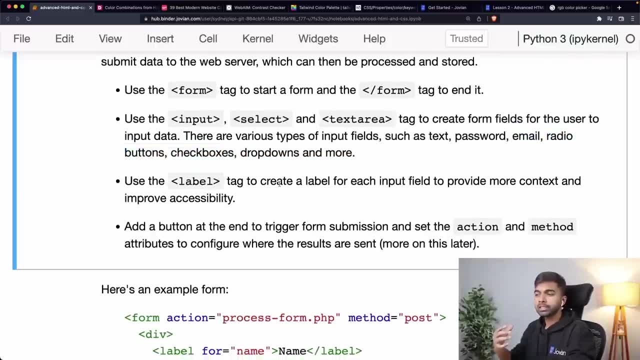 you can have email input fields that automatically validate That what you're entering is an email. You can have radio buttons. You can have check boxes and then, of course, dropdowns, et cetera as well. with each input box of you also have a label. 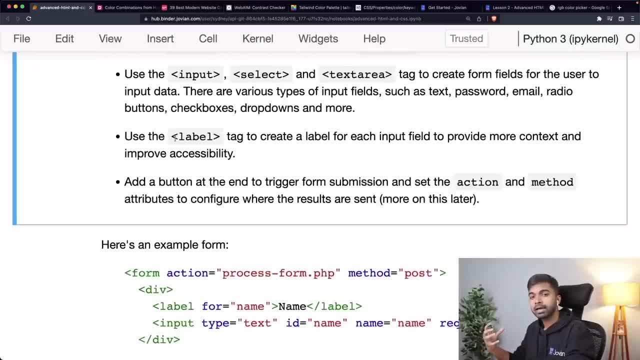 So you have these labels that are associated with these form input tags, And these labels are important because they allow not just the person who's using it normally, but people who are, let's say, who have a poor vision and are using a screen reader labels. 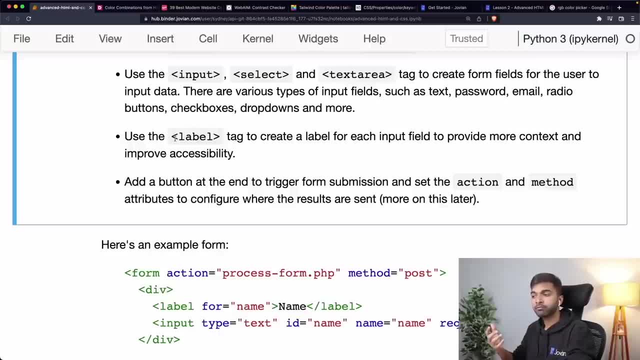 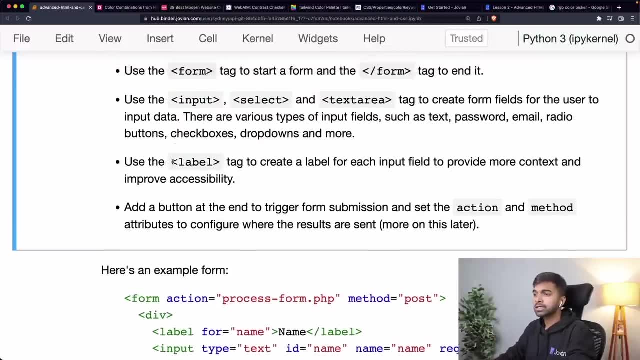 are used. They allow the screen readers to tell people what to enter into specific form fields. Labels are also used by search engines to determine what the structure of your form is. So there are many ways in which labels are important. So don't ignore labels when you're building a form. 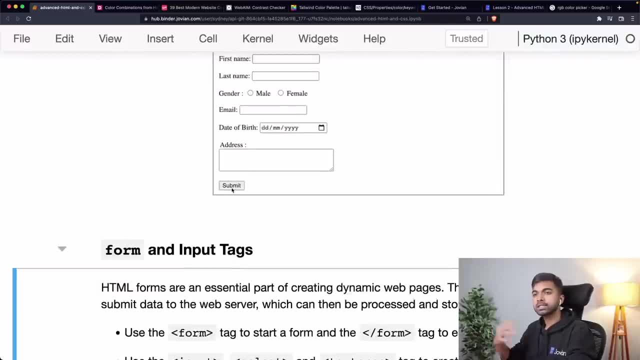 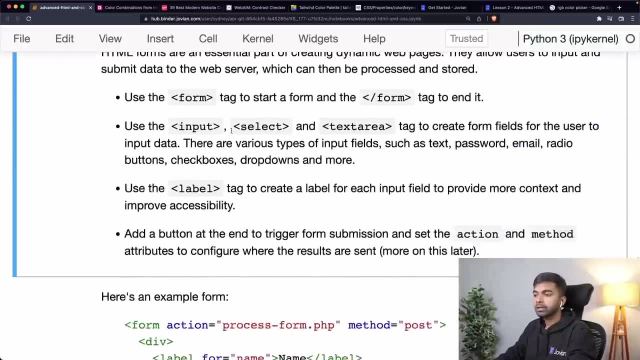 And finally, most forms have a button at the end, sometimes multiple buttons- to reset or clear the data, But you almost certainly have a submit button or a save button or a send button that is going to actually trigger a form submission, which is to grab all the data from the form. 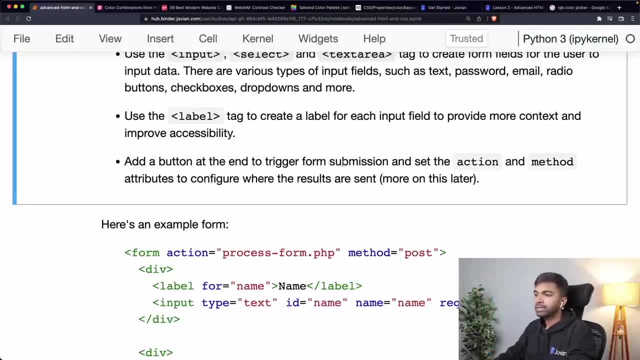 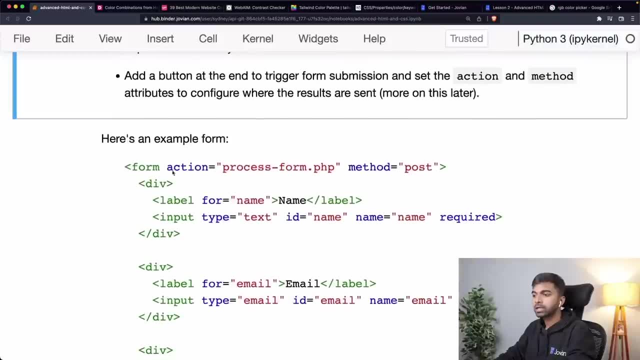 and send it to some server, Some web server, and we send the data using the action and the method attributes of a form. So typically for a form tag, you have an action and then you have a method. Now, of course, in today's lesson we don't actually have a web server, we are just building. 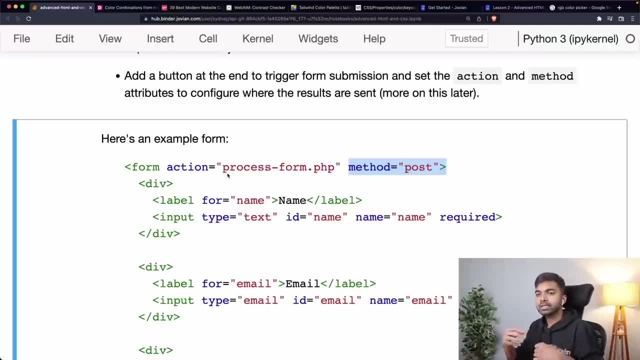 static HTML pages. a server is something that can take some requests, do some processing on it and return a response. We don't have that today, So we're going to be using a third party service to collect these form responses, But over time we're going to learn how to use them. 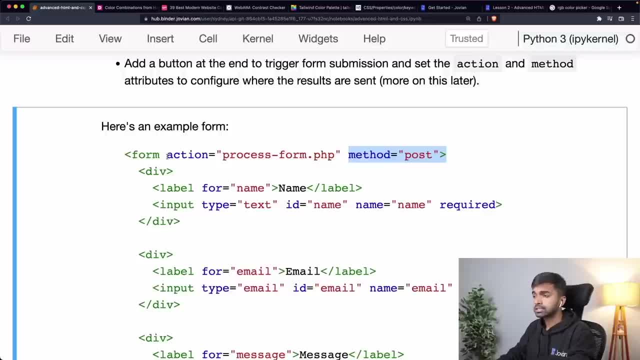 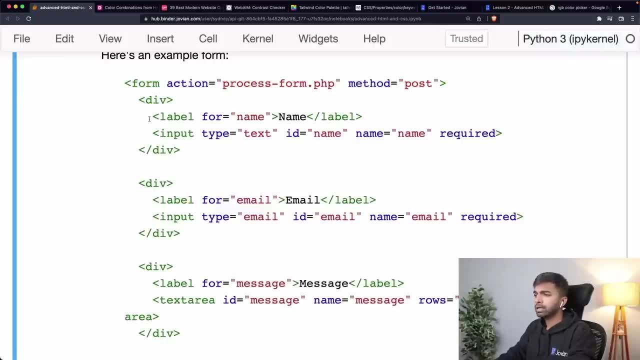 So let's get started. Let's get started. We're going to use our own inbuilt servers. okay, But this is what a form looks like. You have a form here And then inside the form, you can have labels and inputs. 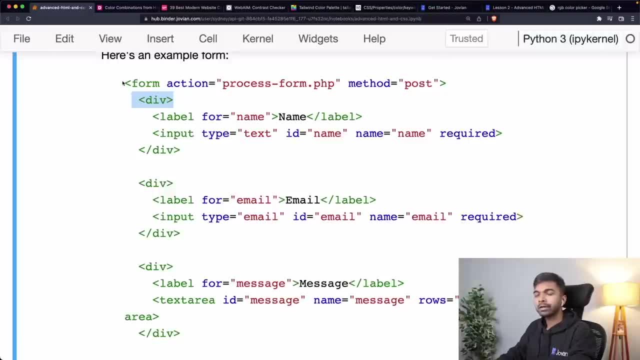 I've put these labels and inputs inside divs, because otherwise you will find that everything just lines up on a single line, which may not look nice. So let's create a form step by step, And in fact we're going to create a form. 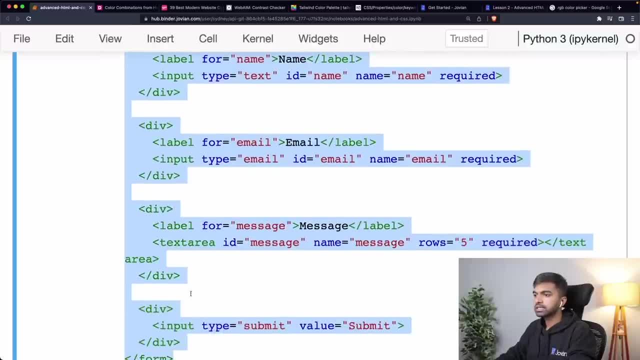 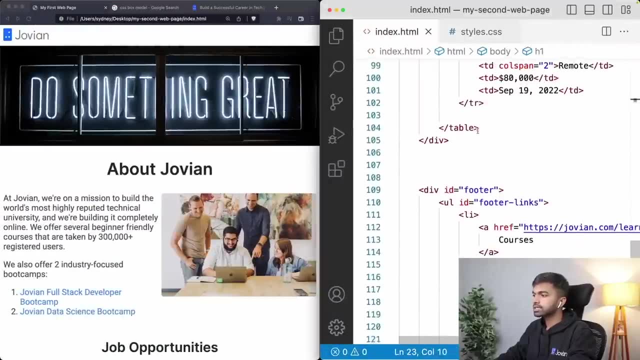 So one thing you can do is you can just copy this code and you can just paste it into the web page And see what that looks like. So let me just show you first, And then we are going to create the form step by step again. 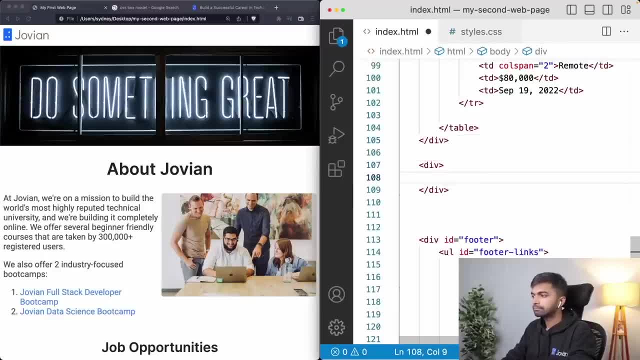 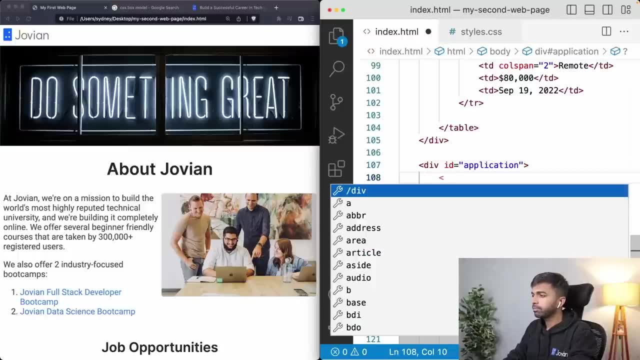 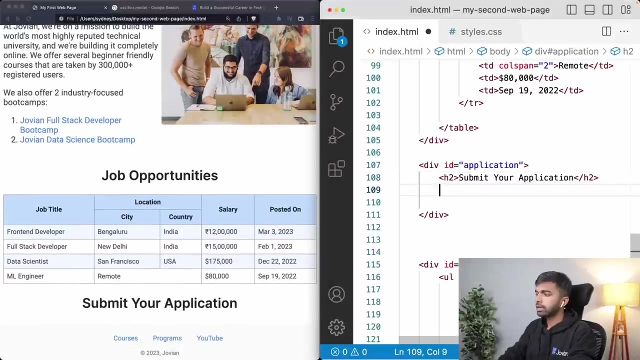 Let me create a div here. first Let me call that application okay, And let me then put in an h2 here and call it submit your application- Okay. So now we have the submit- Submit your application section. Let me then put in this form here: 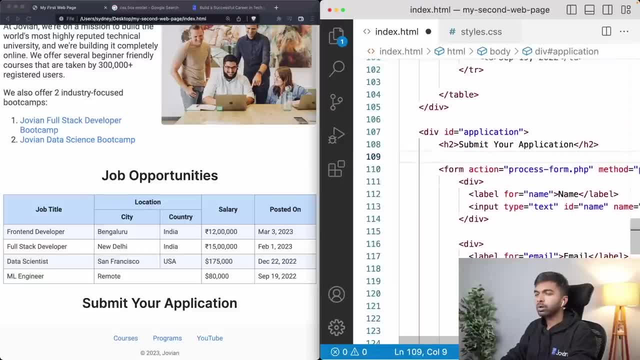 So I'll just paste this form And, by the way, if you just want to include a comment, something that is not actually displayed on the page, you can do that using this comment operator. So started with the open tag and then started with an exclamation followed by a hyphen- hyphen. 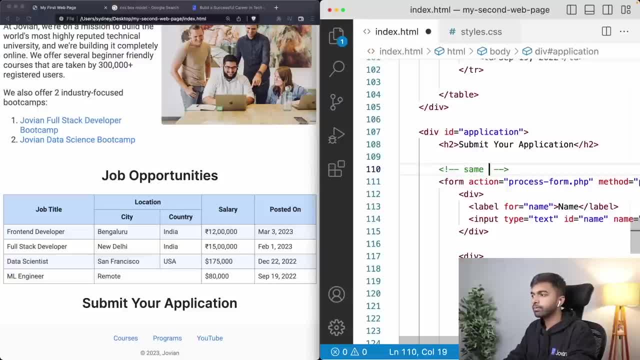 And you can just put some. put some extra system sample form, Remove later. So this is a way for you to just add some note for yourself. This is not going to be read by the browser. this is not going to be displayed on the page. 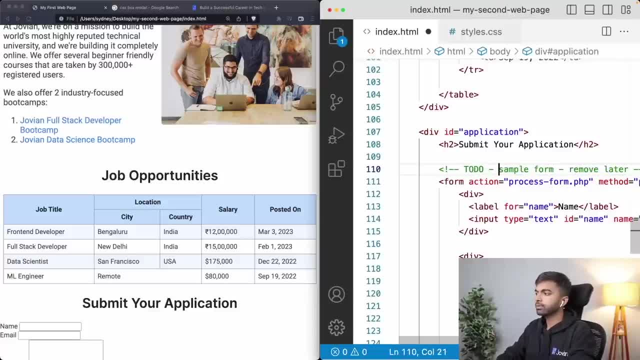 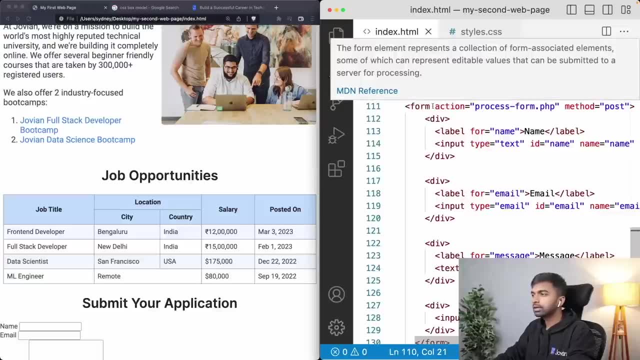 But this is just a note that you can leave for yourself. you can just say: to do and perform, remove later. Okay, But now I've put in this form. So this form has an action, this form has a problem method. These are not things that we're going to use right now. then it has a div. 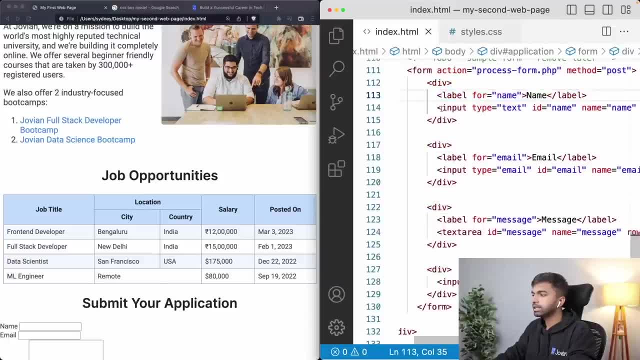 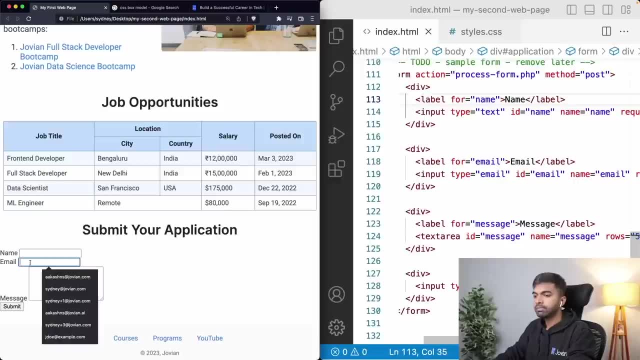 And in this div we have a label, we have the label name and then we have an input And this is what it looks like. So we have name and we have this empty input, Then we have email And then we again have an input, then we have message, then we have an input. 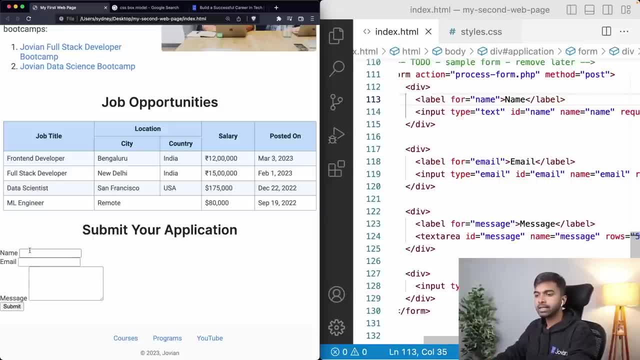 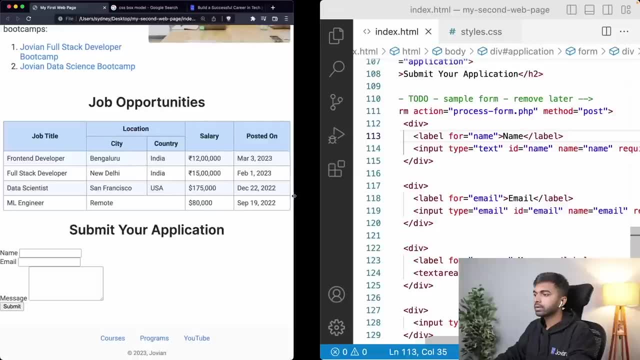 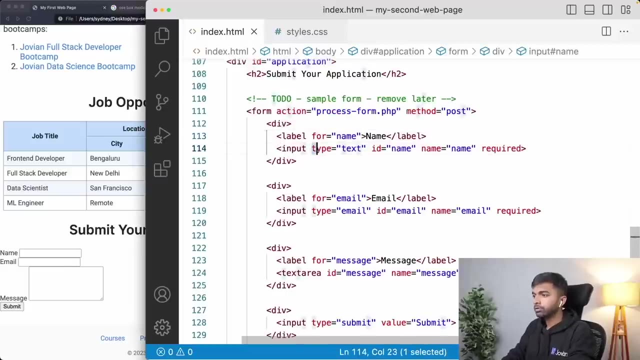 So we basically created a very simple form which contains a label and contains these input fields And a couple of things I want to point out with regards to the structure of the form. Let's make that a little bigger. is that normally, for every input, you have to specify a type? 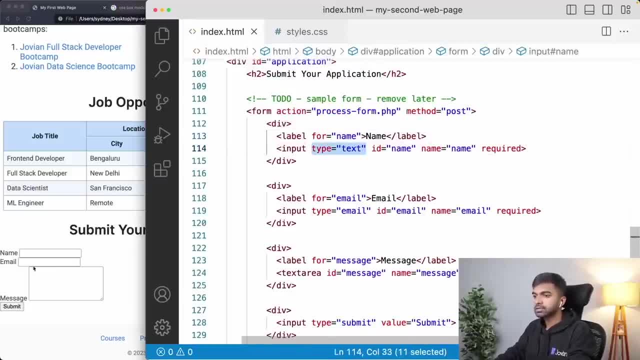 Okay, so here we have specified the type text, So here you can enter any form of text Instead. if you had specified the type number, for instance, then you would not be able to enter normal text here you would have to enter numbers. 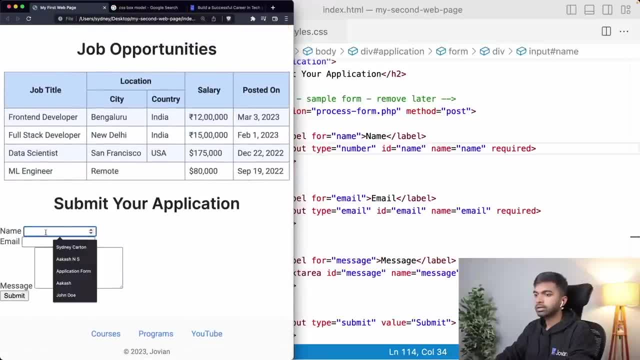 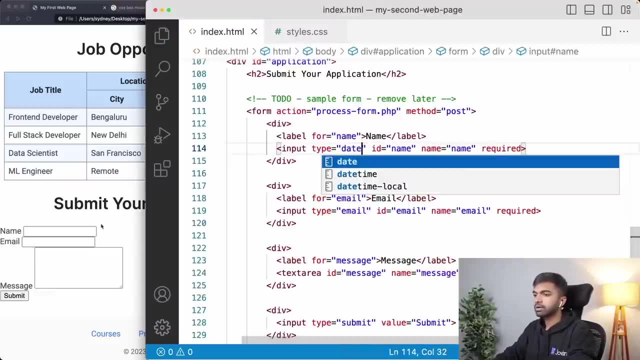 Okay, so that's one thing. I'll just zoom in a little bit here so that you can see that I can't enter text. I have to enter numbers, And you have various other kinds of inputs as well. you have the date input. 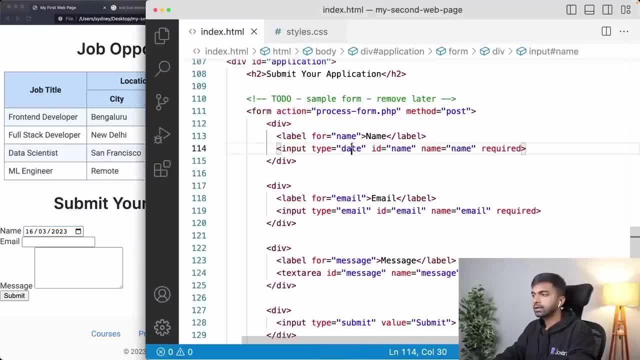 Now, in this case it's going to open up a date picker, So that's nice, But I'm just going to revert this to text for now. Okay, Because it is for name. Then another thing that you often have to do is to specify an ID for each input. 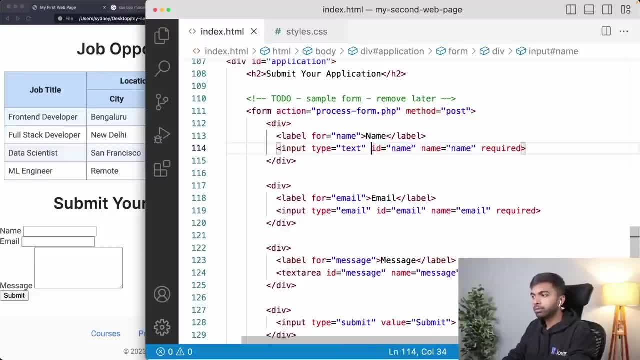 So what is a common practice is to specify an ID for an input and then specify the in the label. which input it is an, it is a label for okay, because the label may not have, may not necessarily always be next to the input itself. 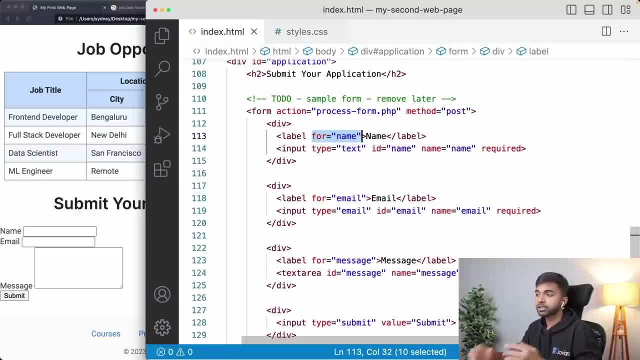 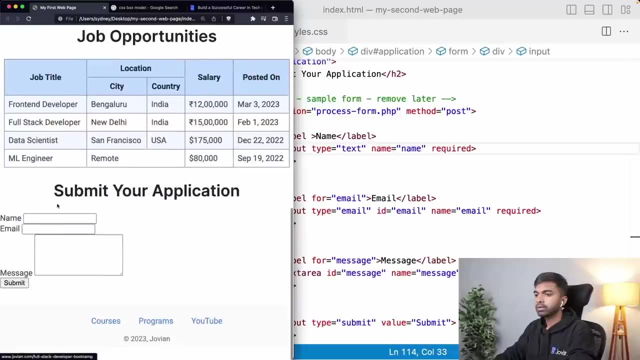 Sometimes the label might be in a different day of the input, might be in a different day because of the structure of the page. So you specify an ID And then you specify that the label is for this ID using the for attribute. your form is going to work perfectly fine without this. you can see that the form still works. 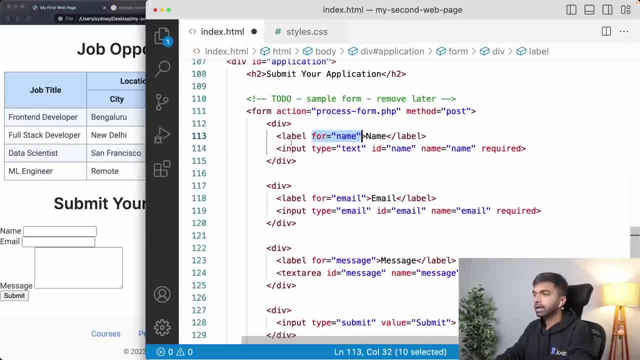 But it's a good practice to specify an ID for the input and specify a for attribute for the label. Okay, so keep that in mind. ID for the input and the ID, of course, should be unique, and the for attribute on the label, which which points to the ID of the input. 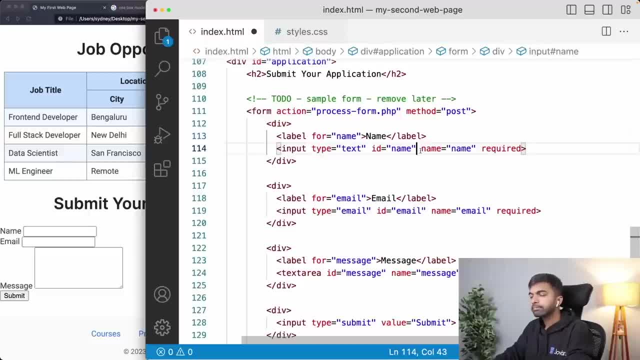 Okay, For which this is a label. Finally, and I know it can get a bit confusing right now, Finally, when you also need to have a name attribute for every input, okay, now, this input itself is also called name. that's a different thing. 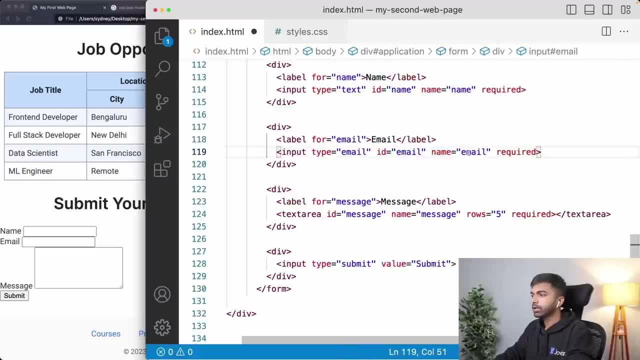 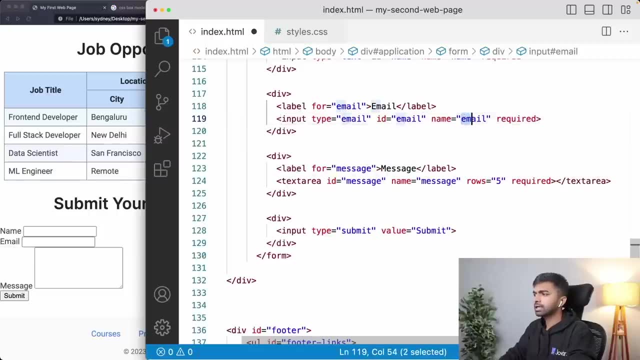 But here is another input called email, and it has the name email, or I could just Yeah. or here there is a- or I could just Yeah. I could just call this something else, Mail ID, for example. Now, what is the value of the name attribute? 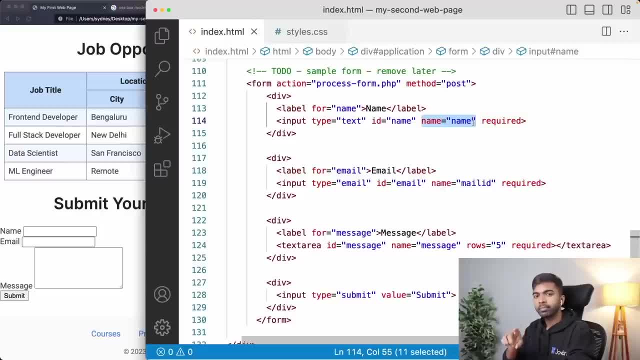 So the name attribute decides that when you hit the Submit button and some data is getting picked up from the form, what is going to be the name of each field? Okay, So if let's say we wanted to send the data to the server in this format? so let's say: 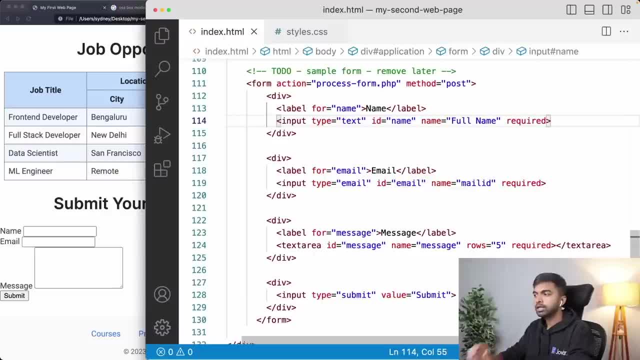 we want to send the data to the server with a full name property and an email address property. So when we click Submit, the server is going to receive the data. Okay, So the server is going to receive some form data And in that form data it's going to have a property called full name, whose value is: 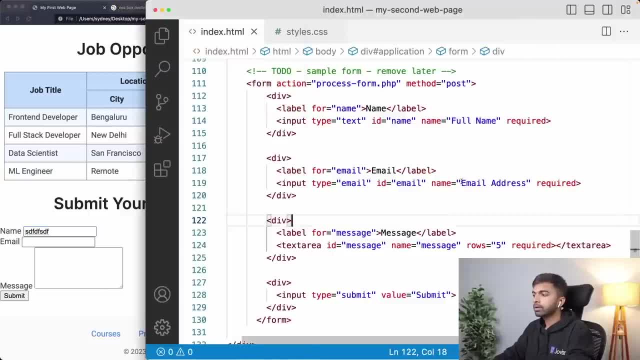 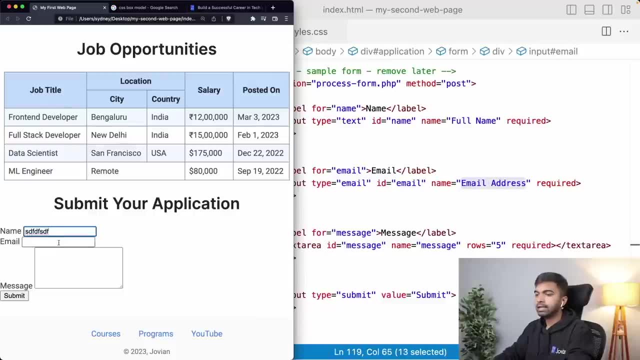 going to be whatever you have entered here. Similarly, the server is going to receive some form data And in that form data there's going to be a property called email address, And that email address is going to contain whatever email address has been put in here. 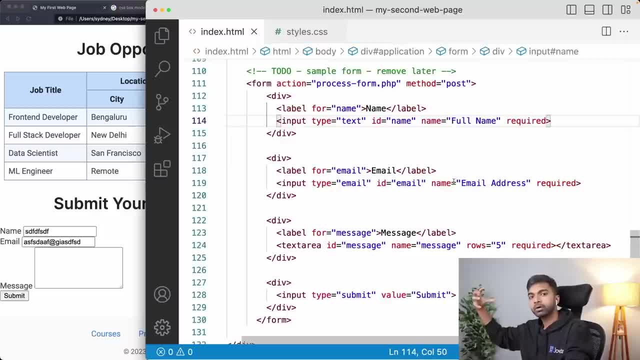 Okay, So the name property is useful on the server Once the form is submitted. we'll see that in action when we actually make a form submission. Okay, And finally, if a form is, if a form field is required, which means it has to be filled. 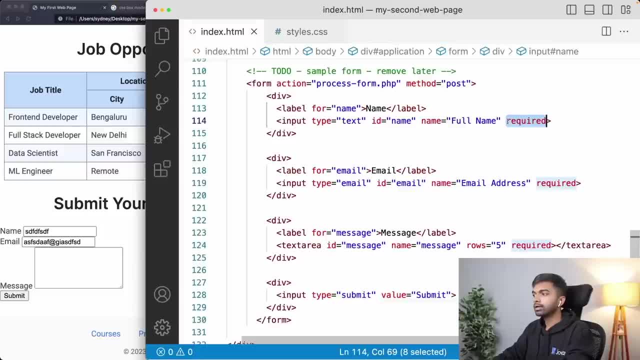 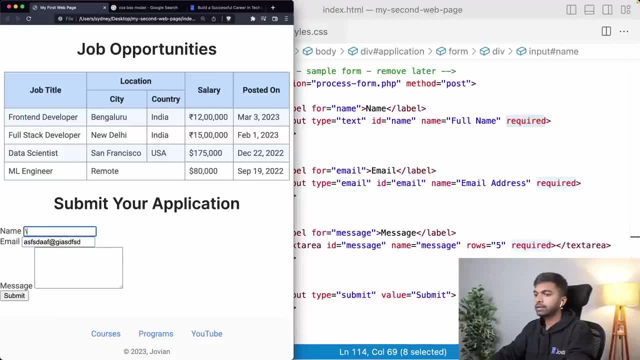 out. without it, submission cannot be made. then you can put in the required attribute here and it doesn't have any value. you just said required And if it is required then as long as you fill it, you will see that you will not be. 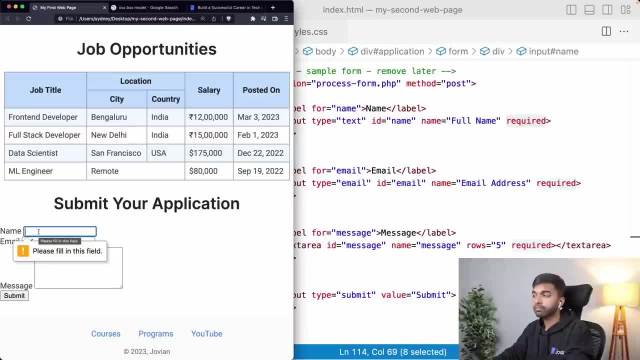 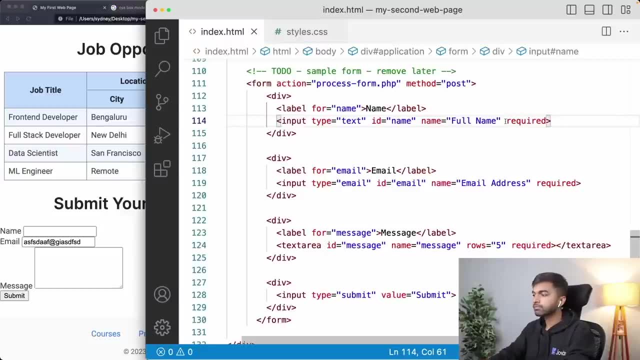 able to submit. So it's just says: please fill in this field when you try to submit the form. Okay, So that is where you have the required property. So those are some of the properties that you can specify for a form Okay. 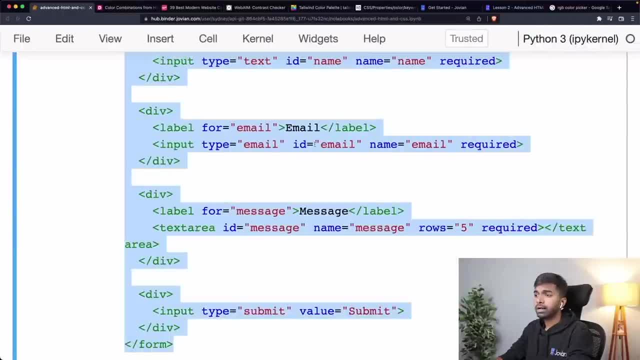 So now we're going to build a form, step by step, for our application. Remember, we had this application form here which has name, email, phone number, position, resume and cover letter. So we're going to build that step by step. 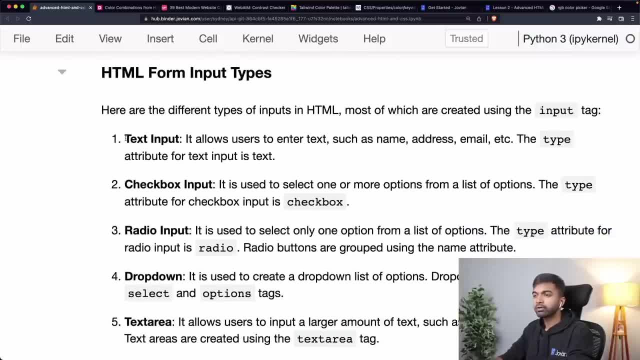 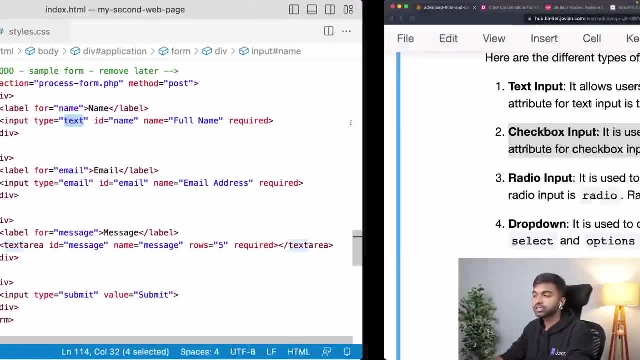 And there are various form input types, So I've just listed a few here that you can browse. you have the text input. obviously we can create checkboxes. So if you just change the type here to checkbox, that is going to become a checkbox. then we 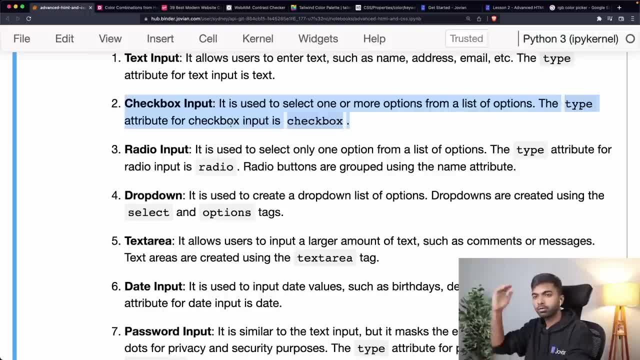 have radio buttons, So checkboxes are often used when you have like you want to show multiple checkboxes. And then we have radio buttons, So checkboxes are often used when you have like you want to show multiple checkboxes and multiple of those can be selected. 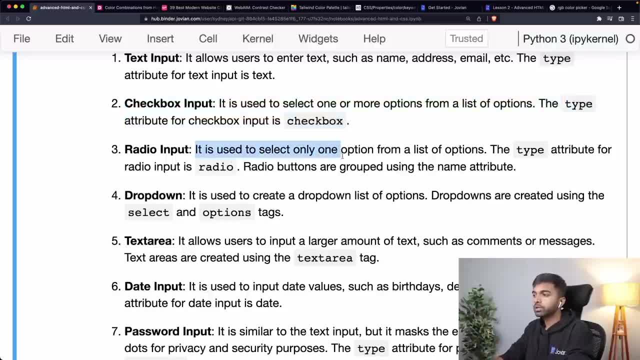 So that's when you show a checkbox, And the radio input is often used when you want to only allow selecting a single option from a list of options. So again, you should experiment with this a little bit. It's all about getting some practice. 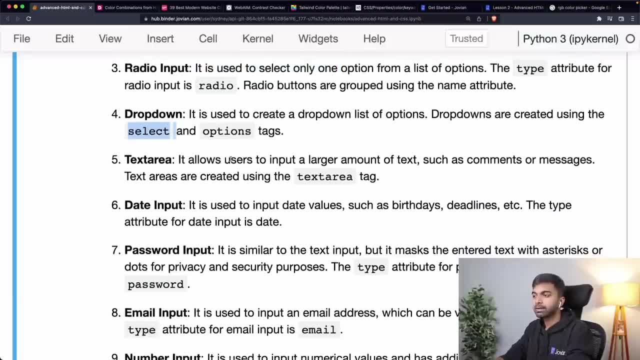 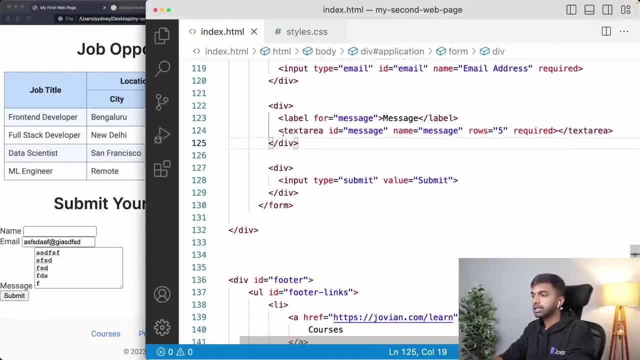 Then, to create a drop drop down, we use a select tag. we're going to look at an example. If you want to allow the user to enter a larger amount of text, then you have to use a text area. Okay Now, one key thing I want to specify about text area in particular is that 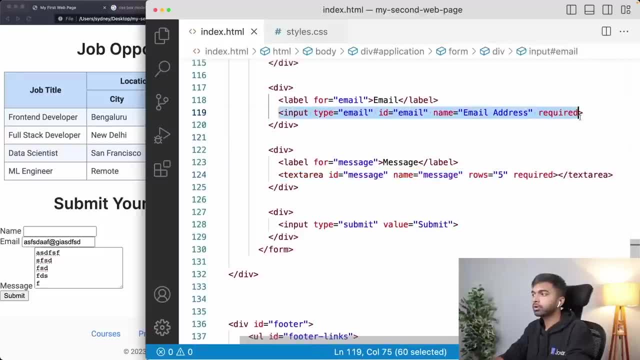 all inputs are generally self closing tags. So the input that you see here, this does not require a closing tag. it is self closing, But a text area is not self closing. So whenever you have a text area, you have to add the closing text area tag as well. 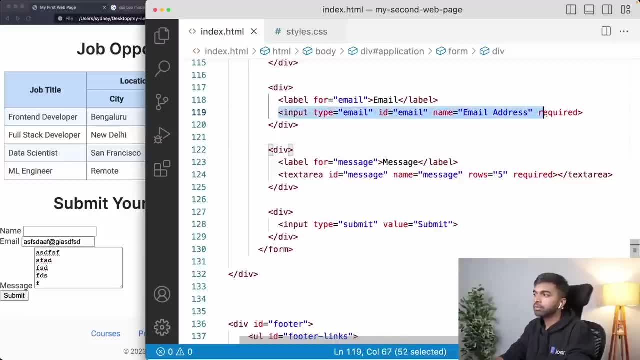 It's just how HTML has been defined. So make sure that whenever you have an input you don't necessarily need a closing tag. you can put one if you want, but you don't need one, And for text area normally you do need a closing tag. 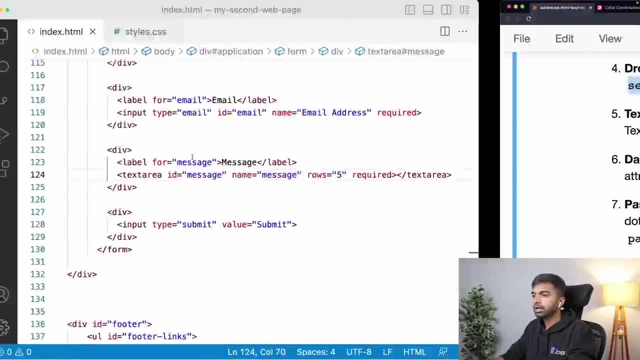 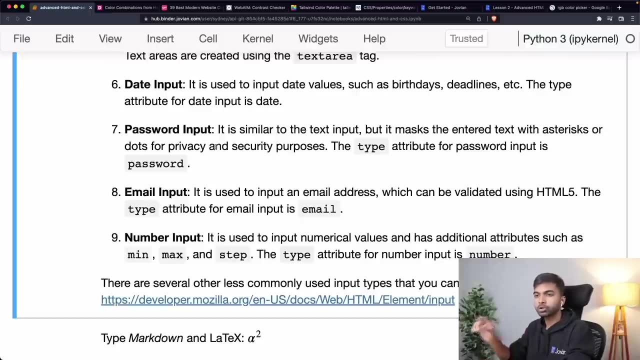 So that's something to keep in mind. Then you can use a date input Again. just change the type here to date and that's going to become a date. you can use a password input in case you want to build a login form where you don't want to show. 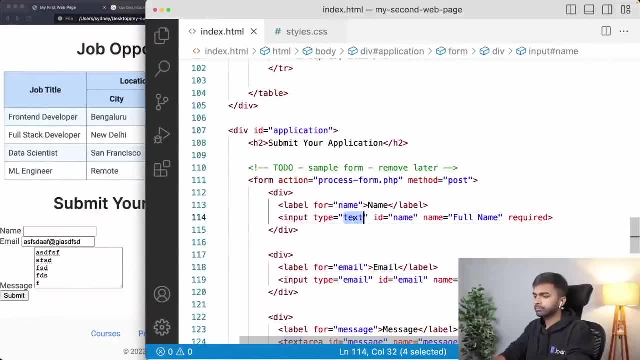 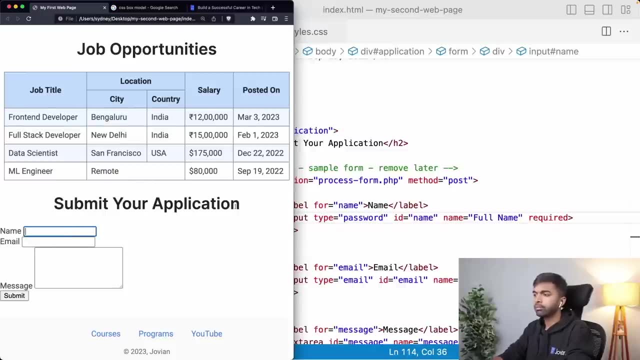 what is being typed. I just quickly show you what that looks like. Let me reload this page. you can see now that whatever I'm typing is not visible here. So that's a password input, And then, of course, you can have email input. 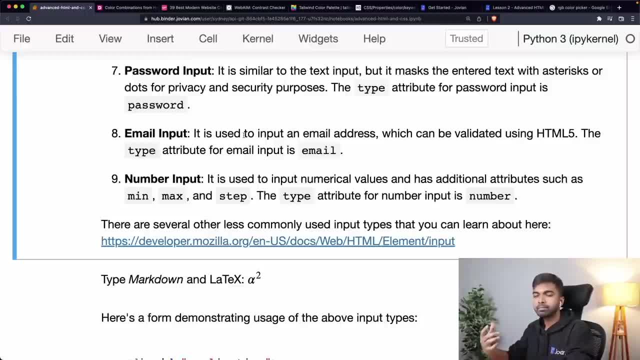 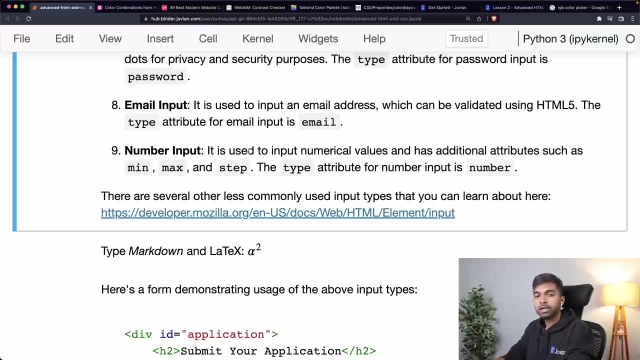 So this is going to validate that the data is being entered, is an email before submission, And then you can have a number input And that is going to make a numeric input field And you can also specify attributes like minimum and maximum And also the step, like, let's say, you want it to be multiples of two or something you 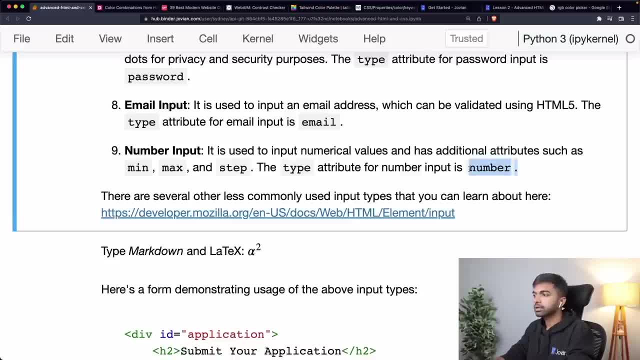 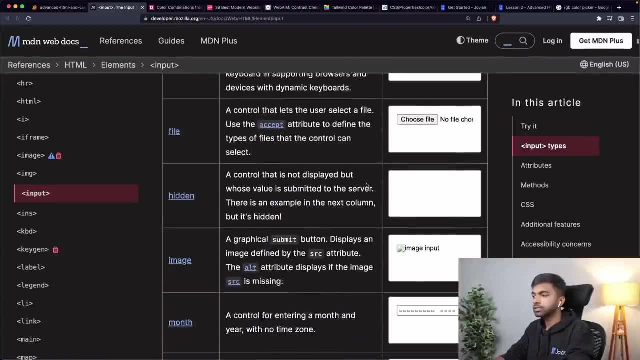 can specify that as well. That is again achieved using the input type. There are several other input tags that you can use, So you can check out various other input types here. there are lots of these. you can have an image input, you can have a color input, you can have a range input, so you can have 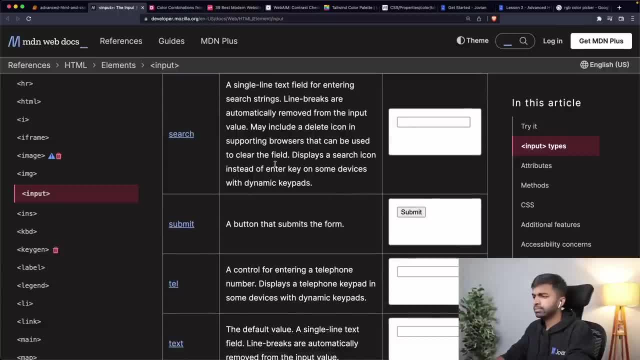 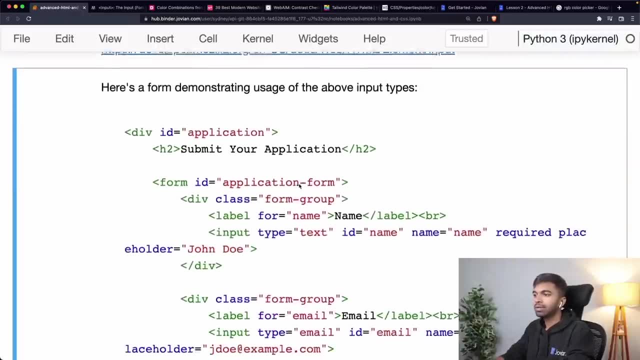 a slider. you can have a search input. You can have a slider, You can have some. submit is, of course, the input that is used to create a submit button. But yeah, there are a bunch of different input types. And now let us actually build out this application form. 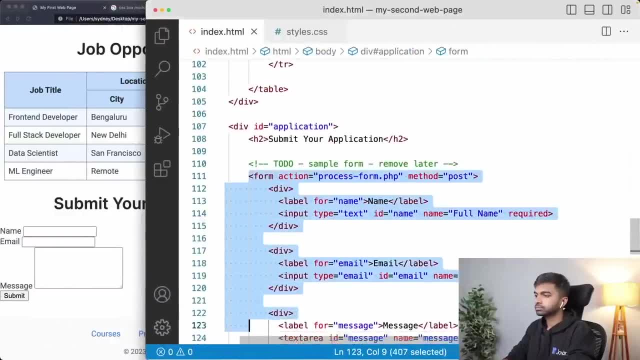 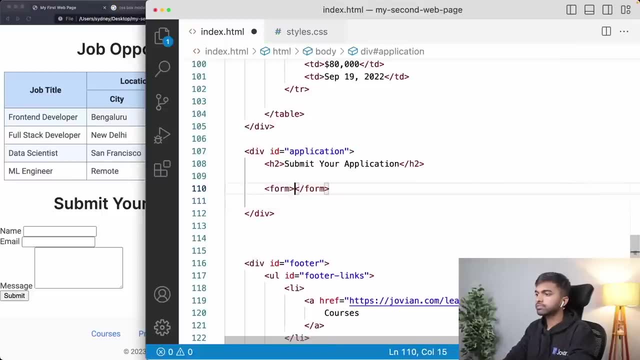 I'm going to take this all away for now And let's start building the application form. So I'm going to just first create a form- nothing- and I'm going to give it an ID. Let's call it application form. And now let us start. 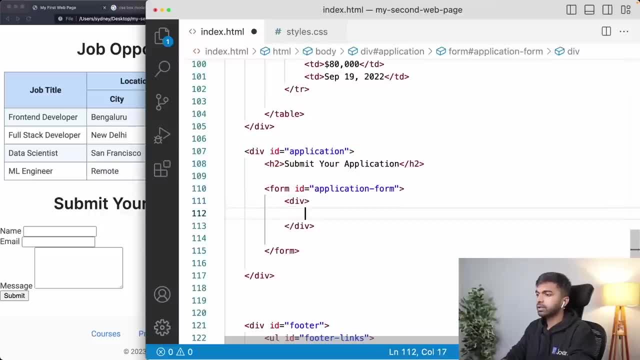 Okay, So let's start by creating a div first. Again, we're putting things in a div so that they just show up nicely, And let us now create a single input of type text And let's give it the ID name And let us give it the name, full name. 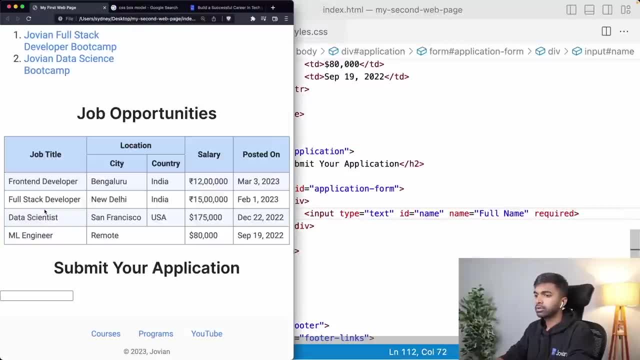 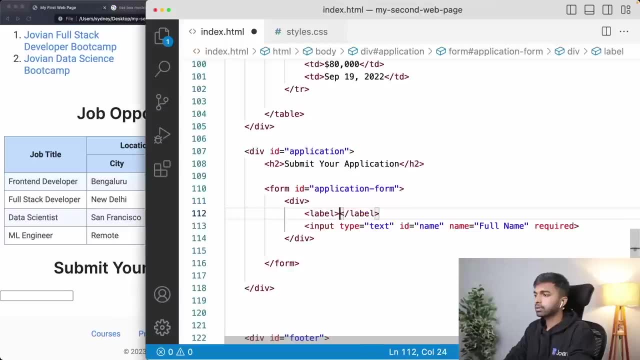 And let us make it required. Okay, And let's reload the page. So now we have this input box, That's fine. Let us put a label for this input And in the label let us put the value full name. Okay, so now we have full name. 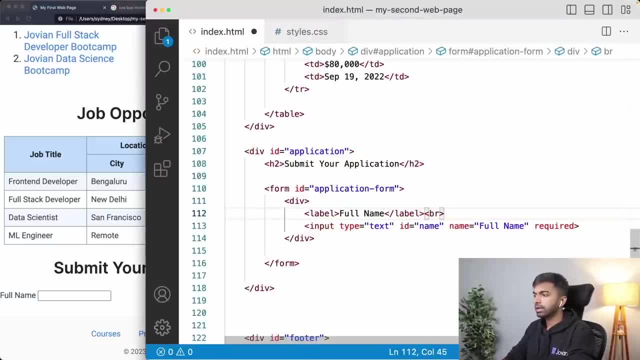 And then we have this box. Let us maybe also add this- a small empty line. So I'm using the BR tag here. it is a self closing tag that is used to add a new line. It's not used a lot anymore, But in forms. if you just want to add a new line after the label, you can quickly add. 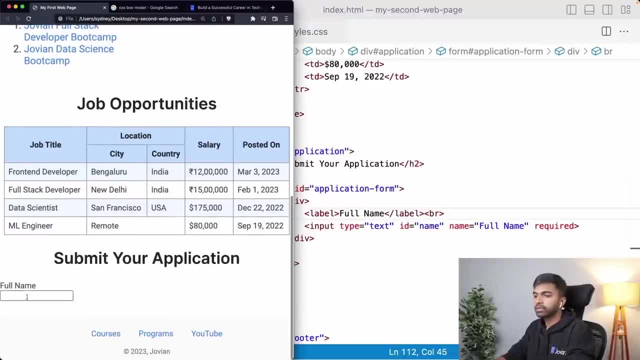 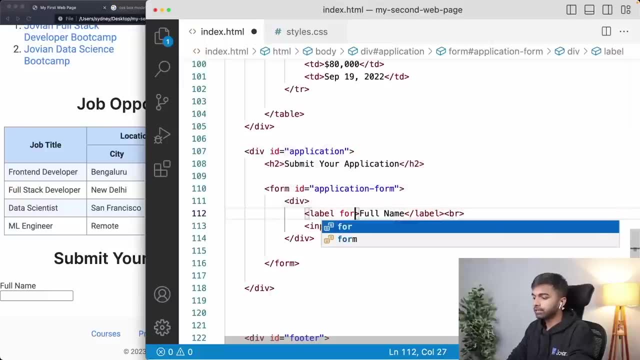 a BR tag, or you can wrap the label in a div. So now this: now you can see that the input box comes below the label. That's one thing, And let us also set the for property that this is for the input with the ID name. 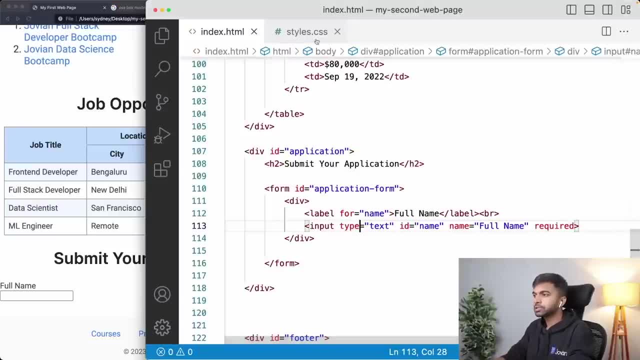 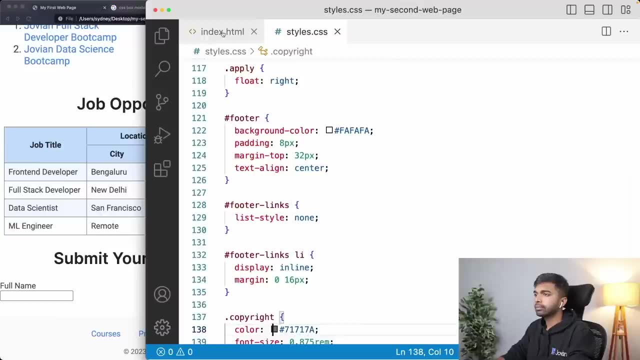 Okay. so that's looking good. The form is looking good. That is also style it a little bit so that it looks slightly nicer. I'm just going to come in here and I am going to first select this application Right now. Okay. 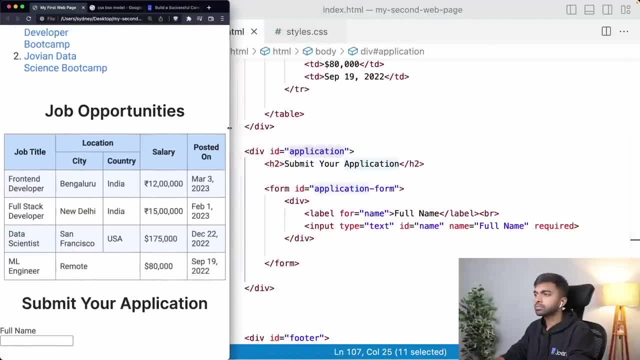 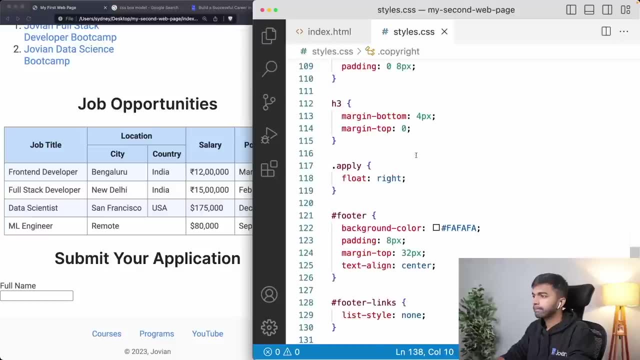 So right now this application div is always at the very left. I just want to make, maybe center it a little bit, So I'm just going to come in here and center it, Let's see. Yeah, let me just add it here. 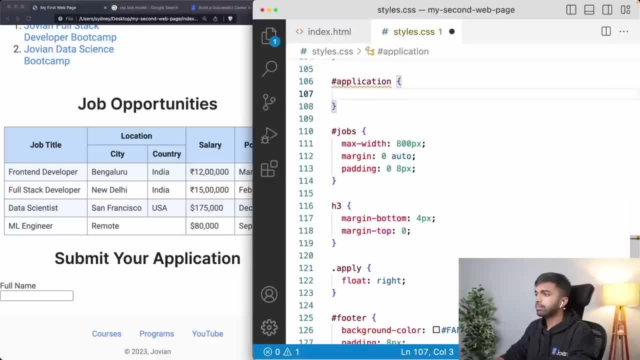 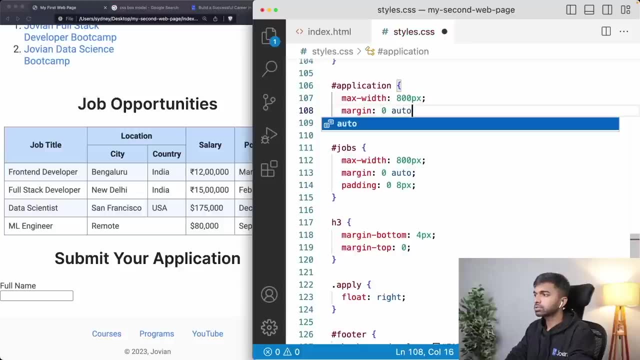 So we have this application div with the ID application. let me give it the same max width of 800 px And let me give it a margin of zero. auto- Remember auto marginal left and right automatically centers the div. And let me give it a padding of zero and eight pixels so that it's not sticking to the end. 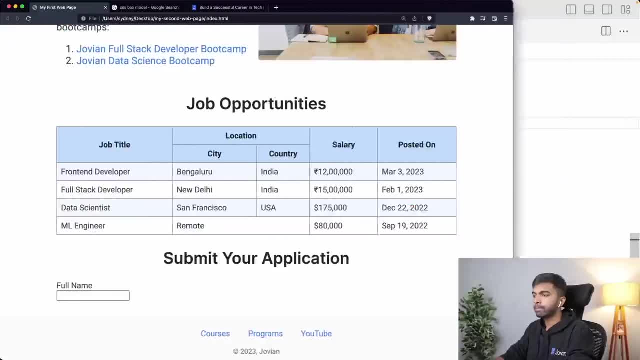 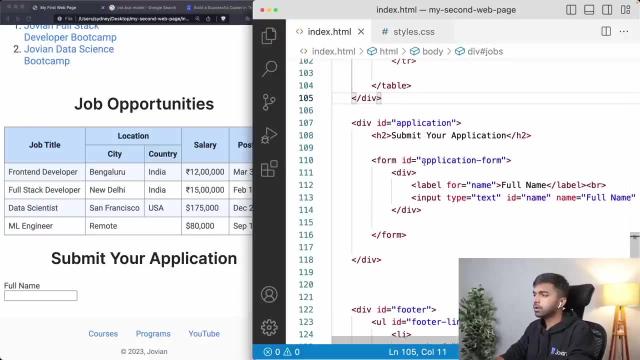 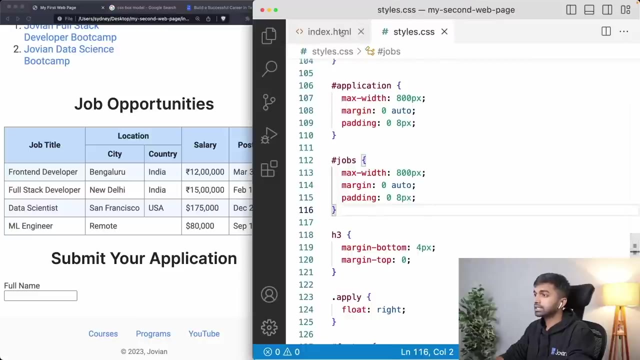 So now you can see here that there's a nice padding, and as I expand it you can see that it remains centered. So that's good. Okay, so far, so good. Then maybe let's also improve the input a little bit. So for the input, actually for the label, 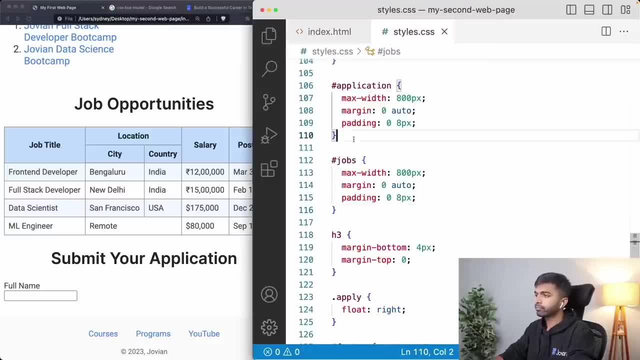 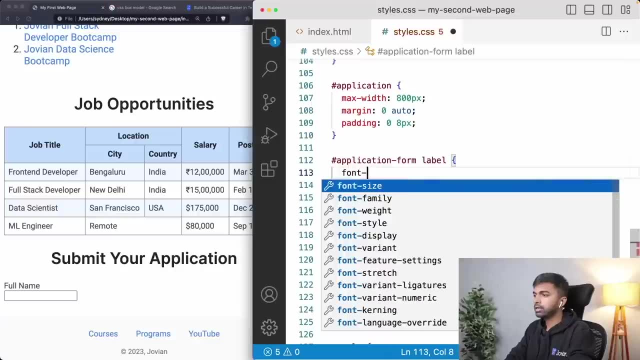 So first let me go in into application div- Application form, Application form, And let me select the label. And for the label let me use font weight: 600 will just make the label slightly bigger or slightly slightly bigger in size. And then let me come in here. 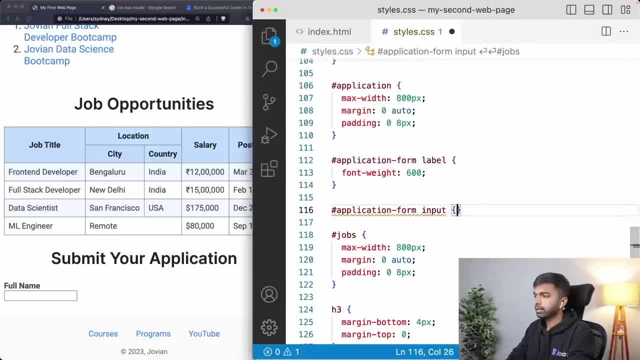 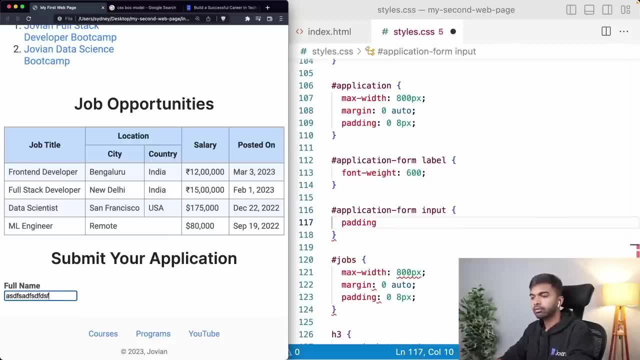 Let me say application form input And let me add a padding here. As I type here, you can see that it's very small. I don't have a lot of space around. Let me add a padding of eight px. Now there is, it's a slightly bigger. let me make that four px. I think four px should be. 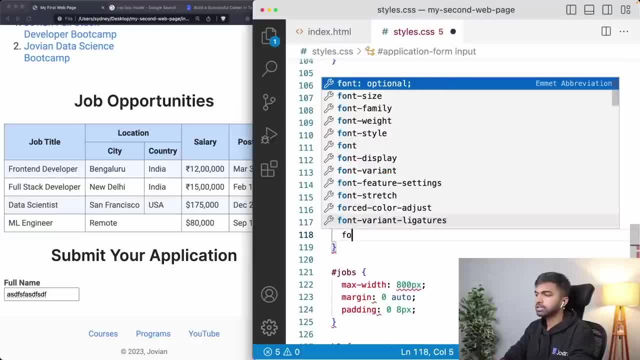 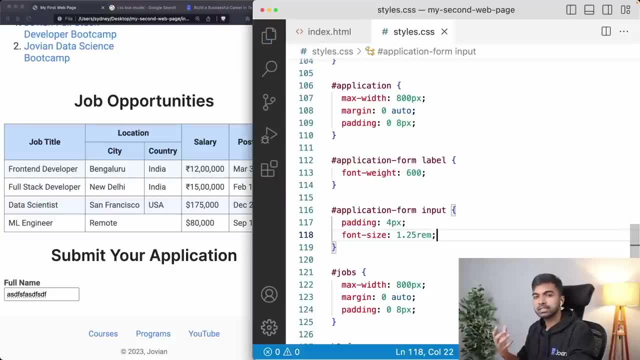 fine, Yeah, so it's slightly bigger. Let me also increase the font size so that the text that I'm entering is of a bigger size: 1.25.. REM, Remember, the base font size is 16.. So 1.25 of that is 20.. 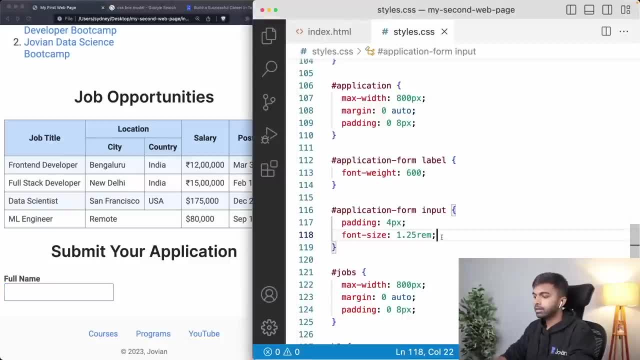 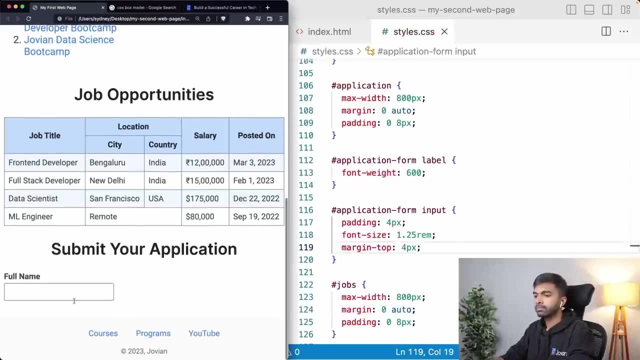 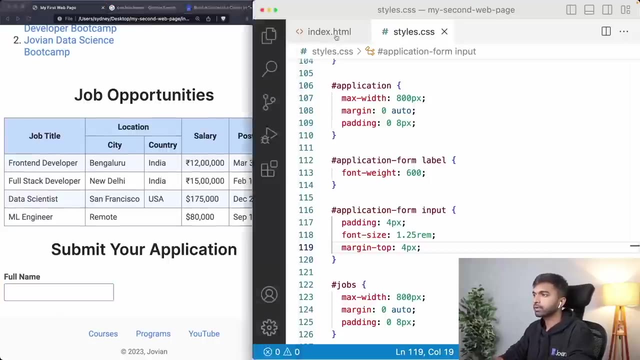 Okay, so now this is looking a little better. And let me also add a margin top here So that it's not sticking to the label. So margin top of four px. Yeah, so this is looking, definitely looking a little nicer. And then I can put in the words Akash and is here and it's starting to look nice. 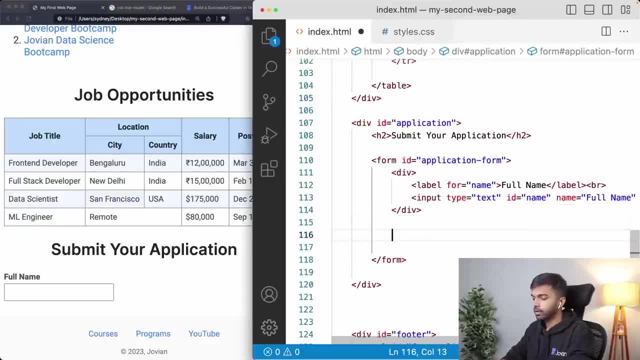 Okay, so that was the input for the full name. Let's then add email And we'll add a couple more and then we start maybe a copy pasting some in the interest of time. So again, label, for I'm going to call the email emails. 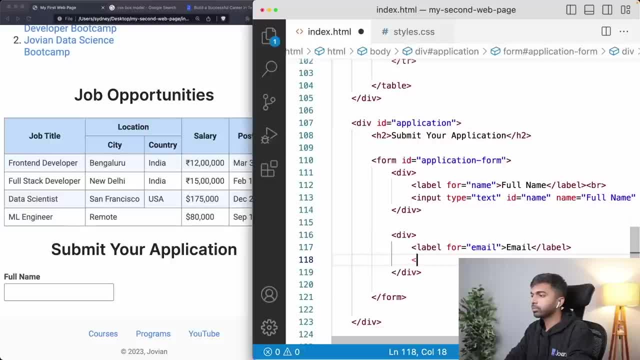 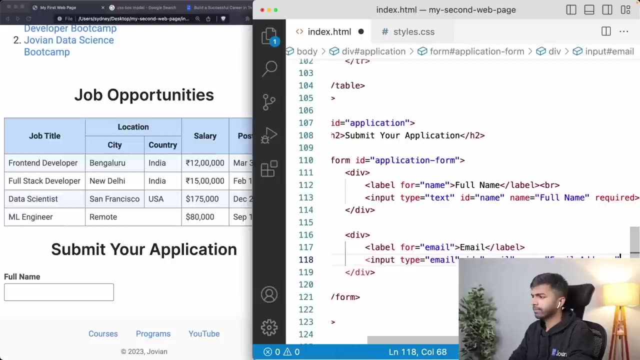 And I'm going to call it email And I'm going to call this email as well, the text that I'm going to put inside the label: input type equals email And ID is email as well, And name equals. let's see email address. 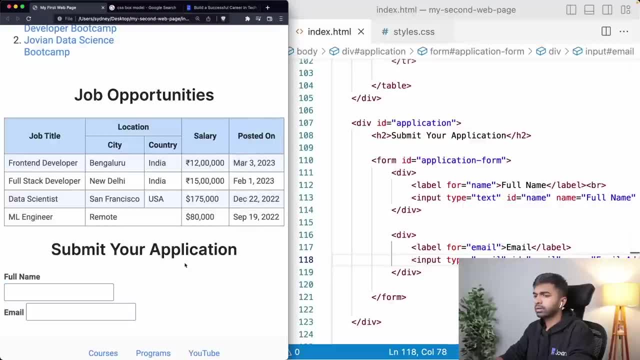 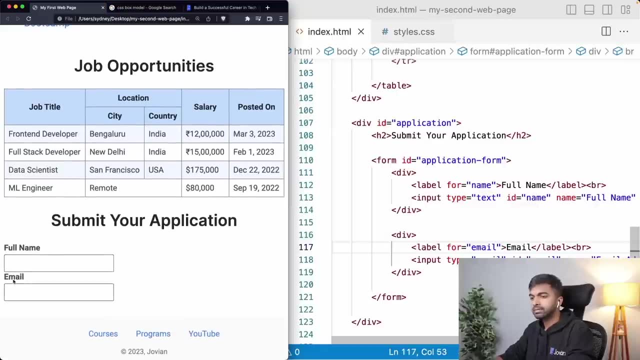 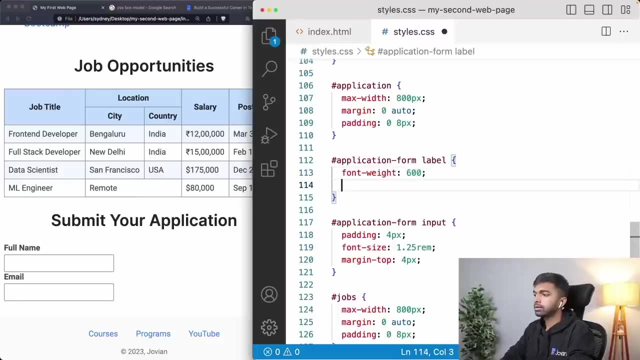 And this is also required. Okay, so now we have email too, And once again, let's add this BR so that this comes on the next line. And I can see that this email is very close to the previous form. So I'm just going to come in here and I'm going to say: label margin 8px, or actually. 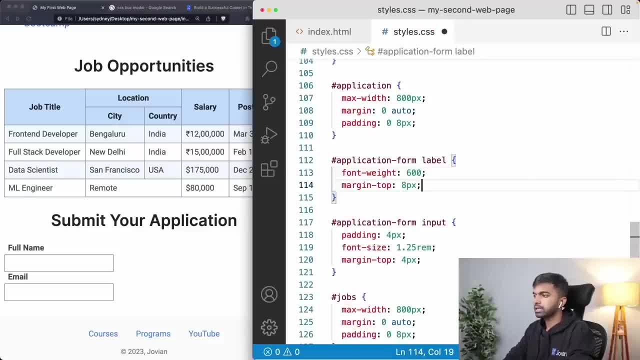 let me just set the margin top to 8px. that isn't doing much. well, let's just set the margin on the div, Okay, Okay. So what happens is that the label is an inline element, just like span, so you cannot set. 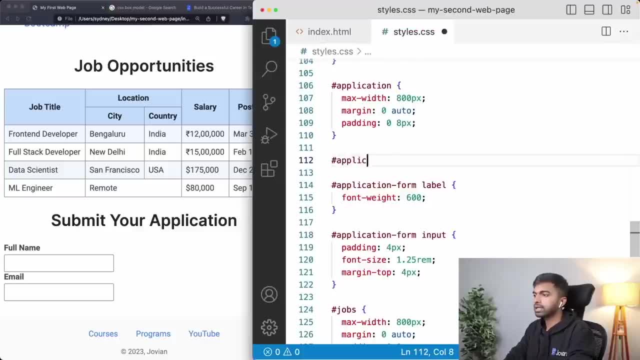 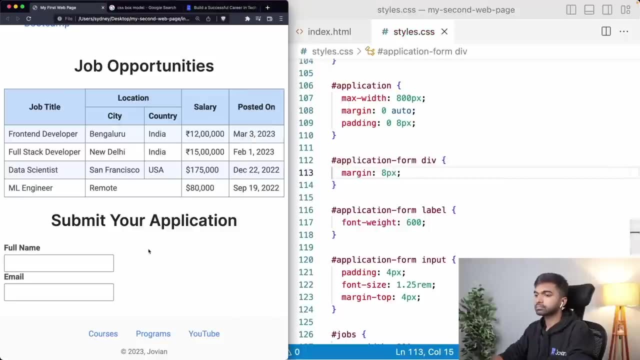 a margin for it. Let's set the margin for the div itself. So, application form: div. let us set a margin of 8px. Now our application form. we could even make this 16 if you want to make it just slightly more spread out. 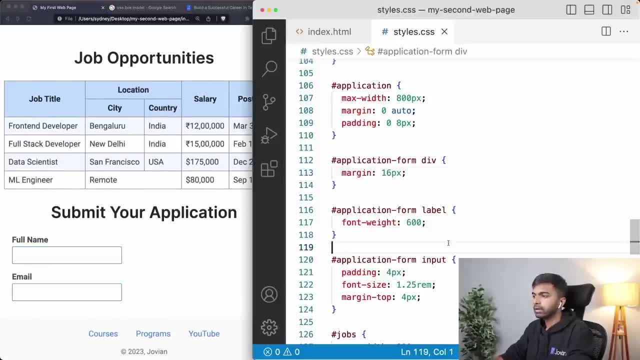 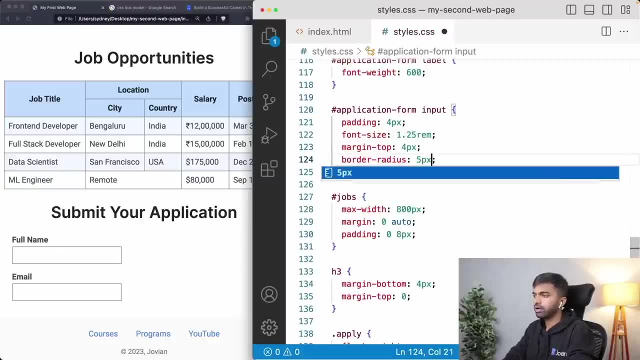 Now our application form is spread out a little better, I think. one other thing that I can do here is in the input I can just add a border radius Of 5px. It's just slightly more rounded and border color of gray, but I could use or I could. 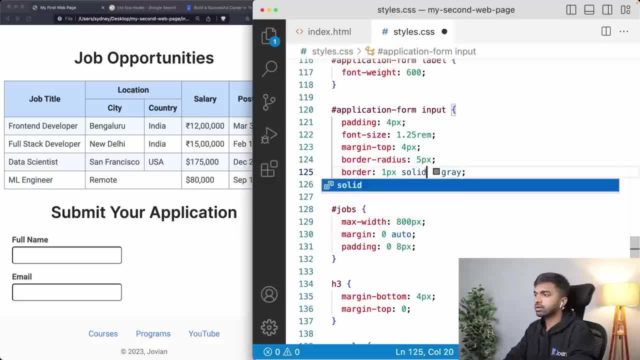 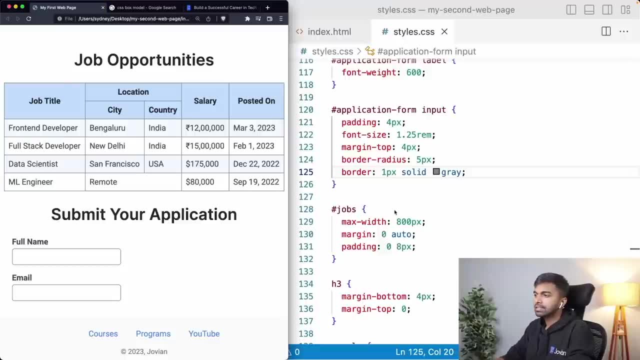 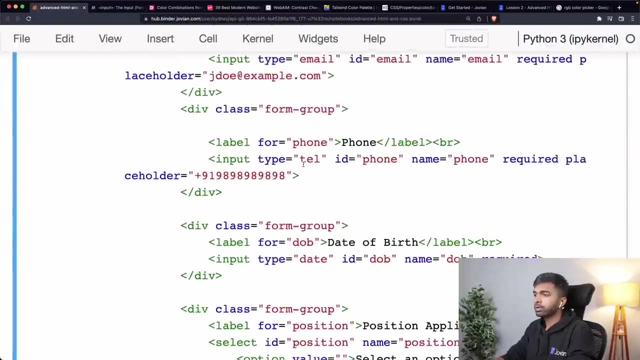 just set border 1px solid gray, And now it's looking slightly nicer. Okay, So we just slightly making these a little nicer. Let's add, maybe what next? So we wanted to have the phone number, So let's grab the phone number here. 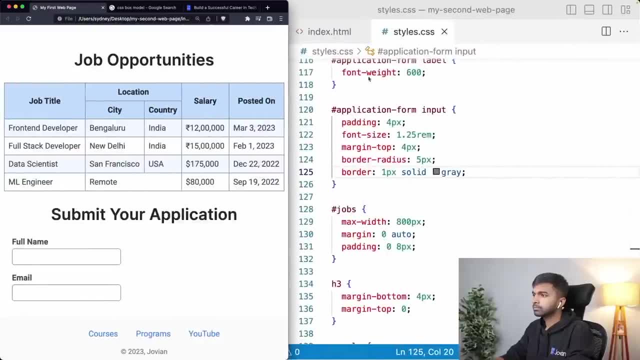 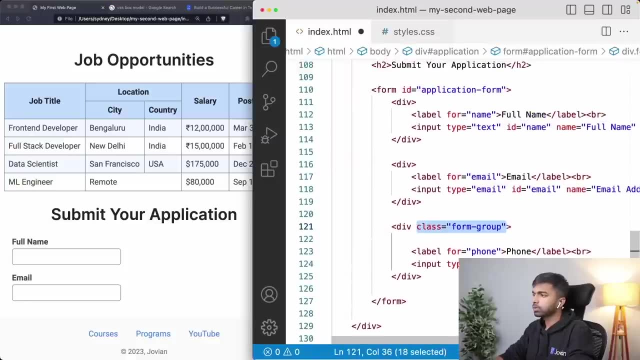 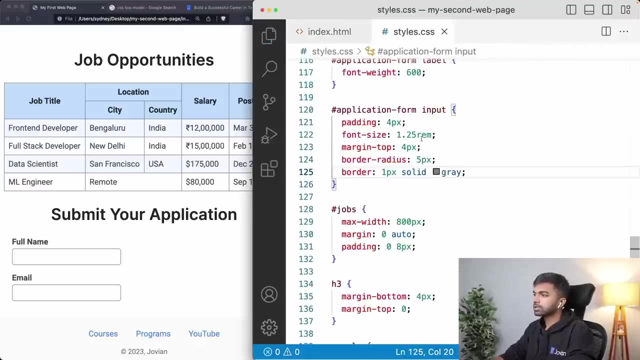 Okay, So this is the class for phone number. And yeah, I think we can add this form group class to select the divs more easily. I'm just adding the class form group for the div so that I don't need to select it, like. 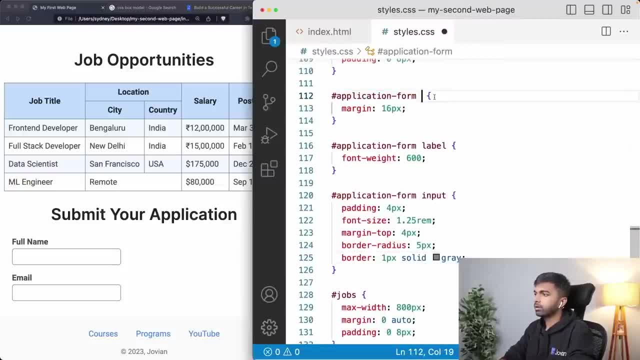 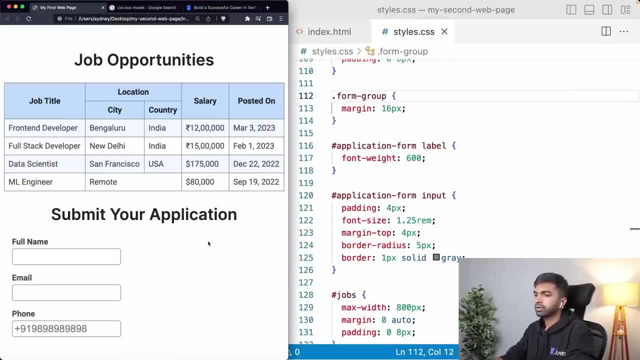 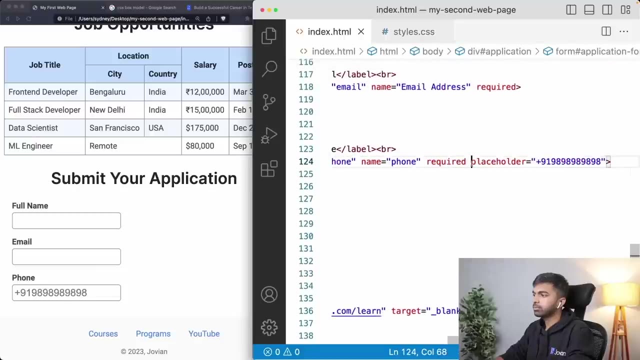 this I can simply say: dot. form group: Yeah, Okay, So now we have the phone number. Okay, So now we have the phone number and you can see here in phone number we've actually added a placeholder, So we've added this thing called a placeholder. 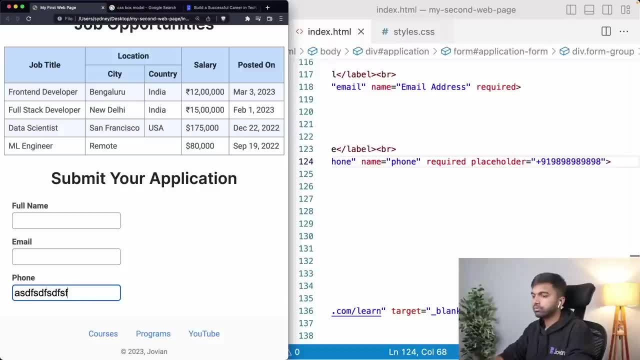 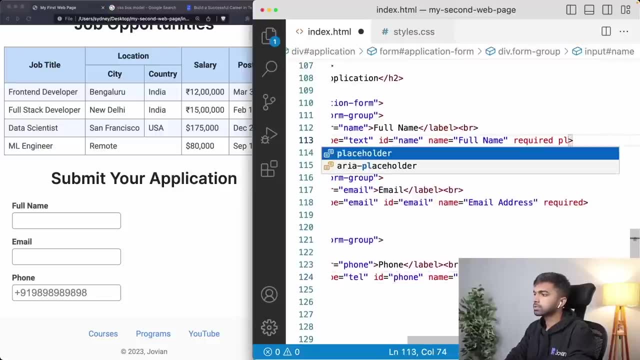 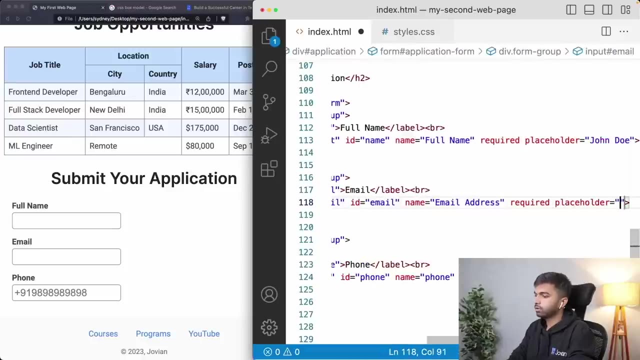 What it does is it fills out an empty value that goes away when you try to fill something inside it. Okay, So I am going to come in here and add a placeholder for the name as well, So placeholder equals, let's say, John Doe, and I'm going to come in here and add a placeholder. 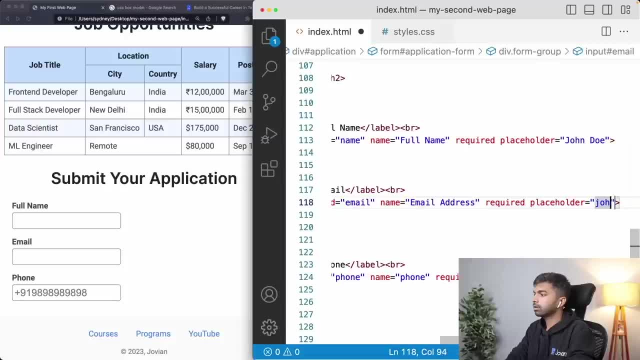 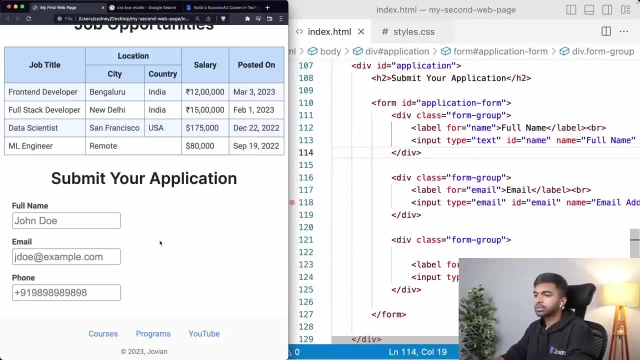 attribute for the email as well, Let's say John Or J Doe, Okay, Okay, So I'm going to add a placeholder at examplecom. Okay, So these are all various attributes that you have to specify. Now we can see that we have this placeholder. 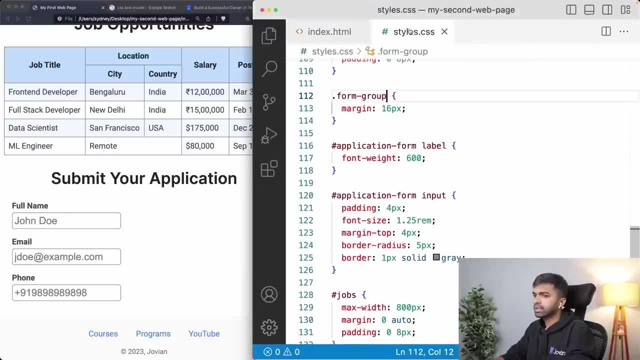 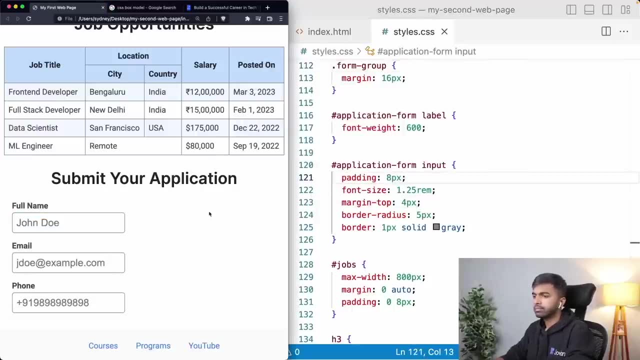 So this is looking nice and let's see, maybe make this. adding a little bigger, maybe eight pixels look even nicer. Yup, Okay, What next? Next we have the date of birth, which is a date. Let me add that in here as well. 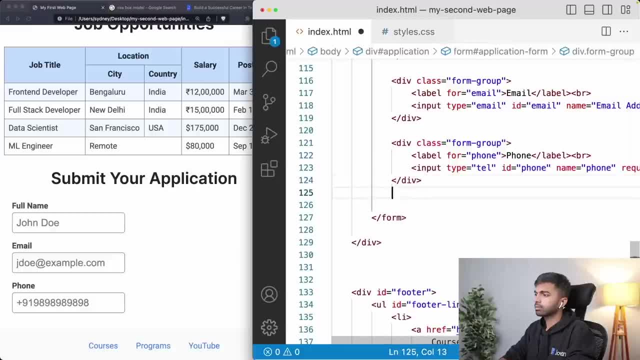 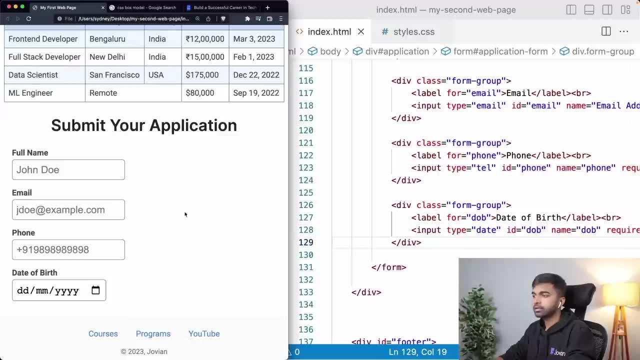 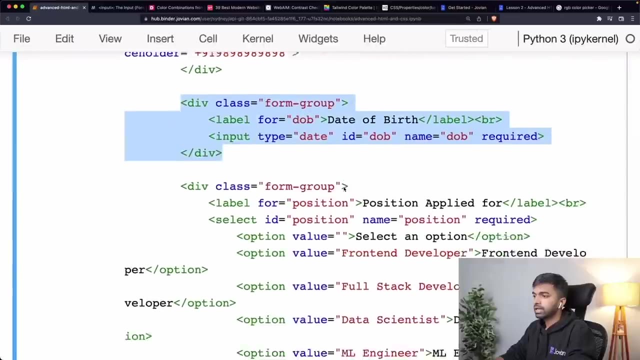 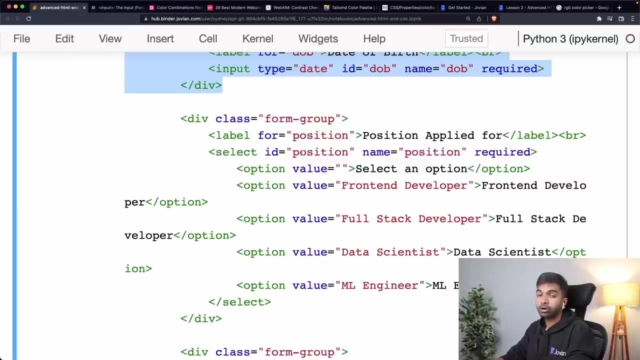 So now we are adding the date of birth. Okay, Now date of birth automatically gives us this nice date selector. That's nice. We can also specify max and min property for date of births, in case you need that. What next? So next we have this position applied for, which is a dropdown. 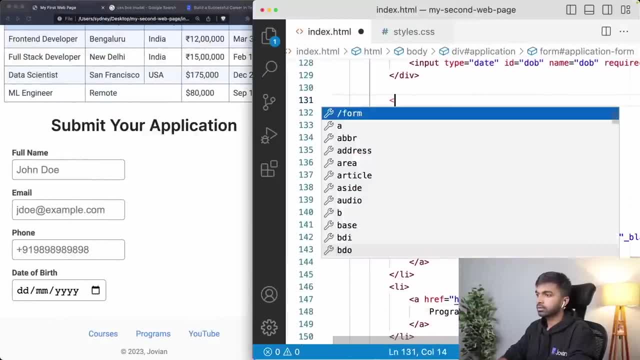 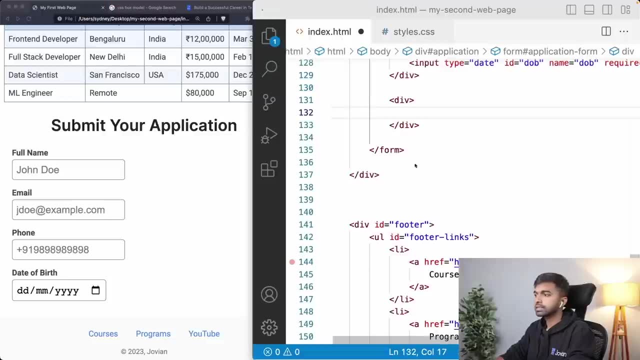 So here's how we create a dropdown. So we go in here And Let's see: Yeah, we go in here and let us create an input, let us create a label and let's say position applied for and let us give it: or equal to position. 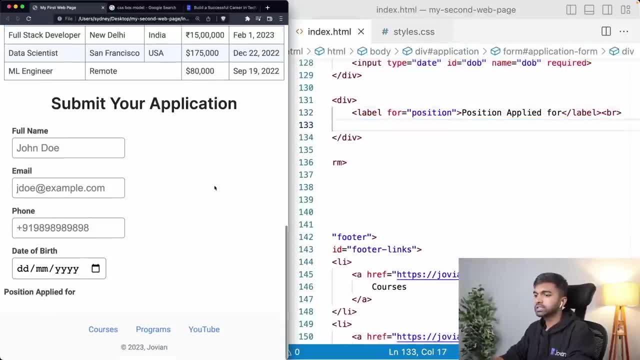 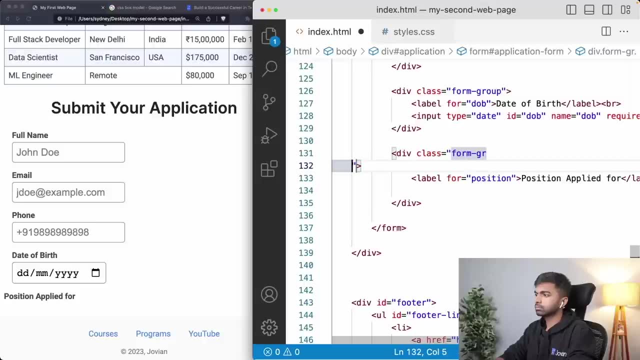 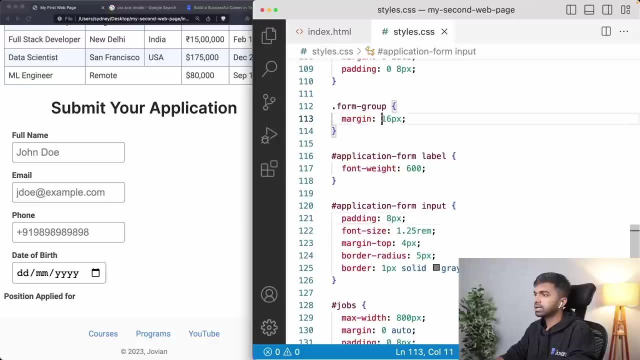 Let's add a BR here, Okay? So now we've just added the label and let us also give it the class form group, And maybe I don't need a margin all around. Maybe I can have a zero margin at that. I can have margin just on the top and bottom and the left and right margin can just be. 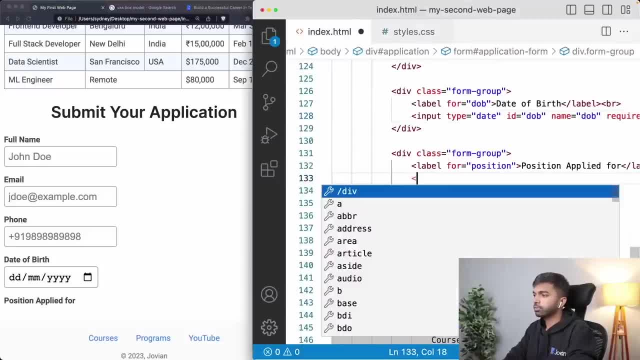 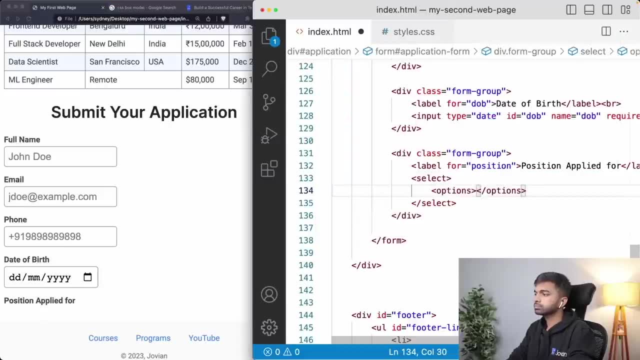 zero: Okay, So we have the label position form group. Then we create the select- Okay, So we put select and inside select we put options or option. So what are the options we have? We have a front end developer- Okay. 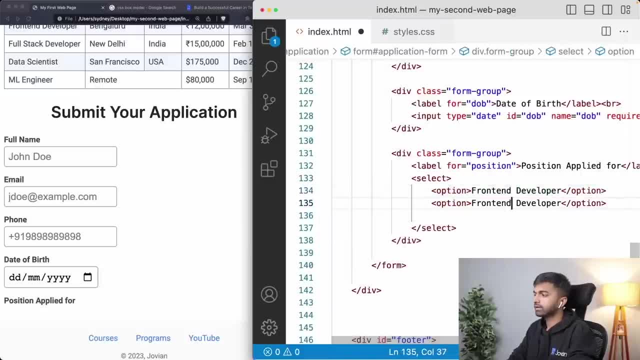 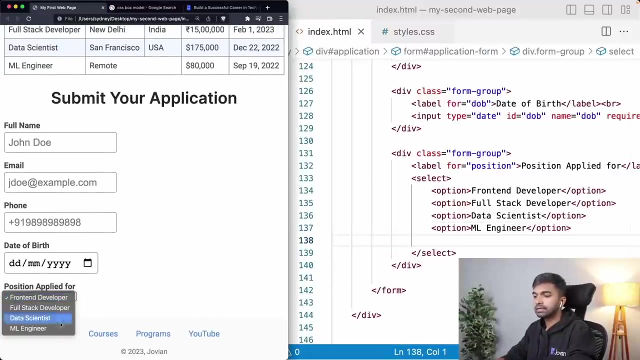 We have a full stack developer, We have- let's see- a data scientist, and we have what else? We have a ML engineer, right? So these are the options. Now we have this nice select which has these options. Of course, we may need to style it as well. 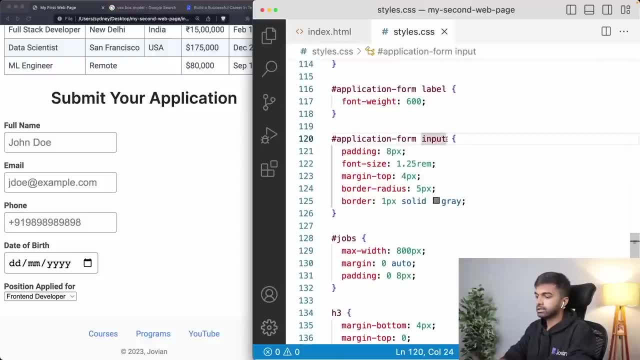 So, again, one trick I want to show you Here is I want to apply these not just for input, but I also want to apply these for select. I'm just going to add comma select and that automatically gives me this. 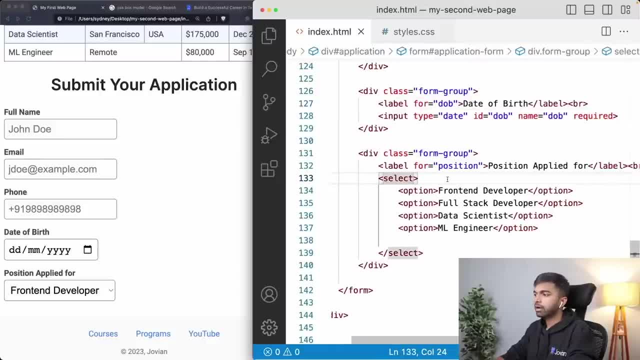 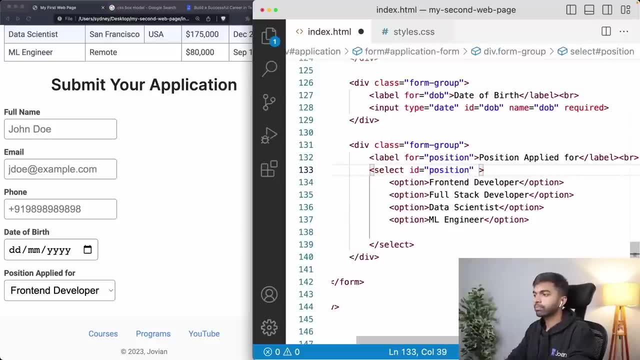 Okay, Now I want to show, I want to tell you a few things you need to have in select. You need to, of course, have the ID, so that the position is not compulsory but it's good to have, so that the label is specified properly. 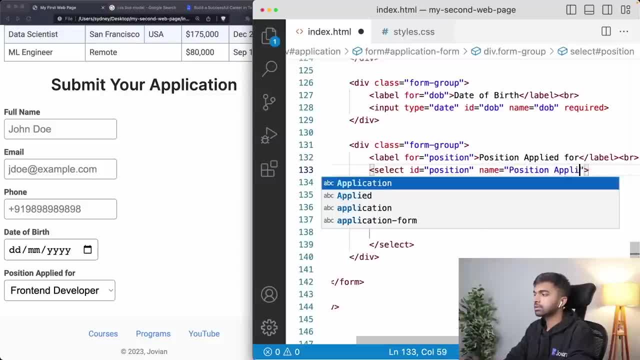 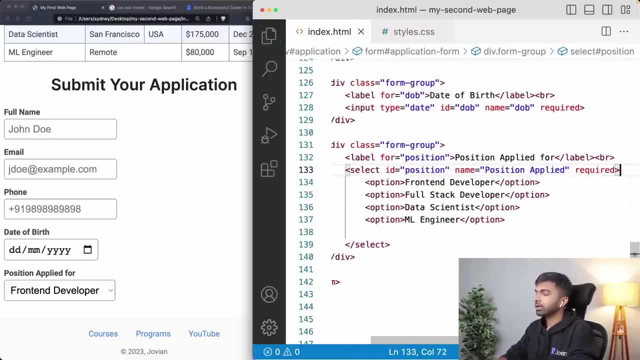 Then of course, you need to give it a name. So then in the name I'm just going to say: position applied. That is what is going to be sent to the server. Then what else Is it required? Yeah, I want it to be required. 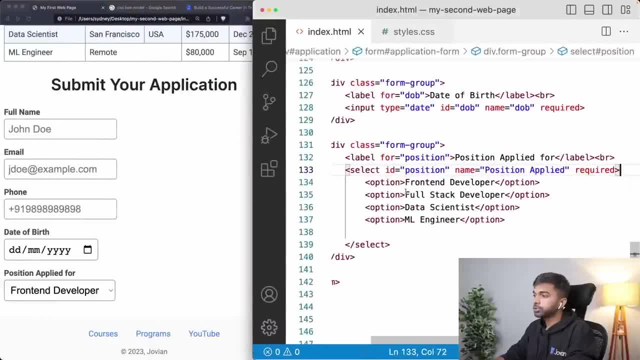 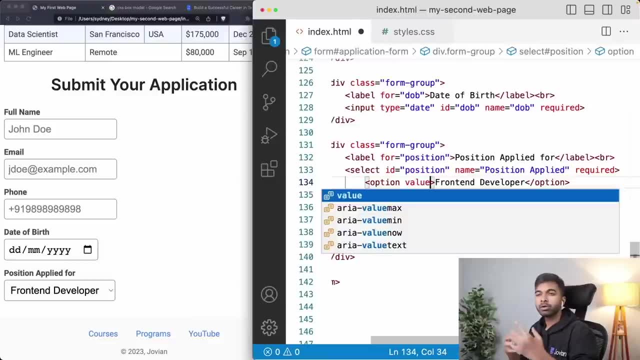 What else do we have here? Yeah, So for each option you need to specify a value. So what ends up happening is what you show on the screen and what is sent to the server, maybe two different things. So for each option you have to specify a value. 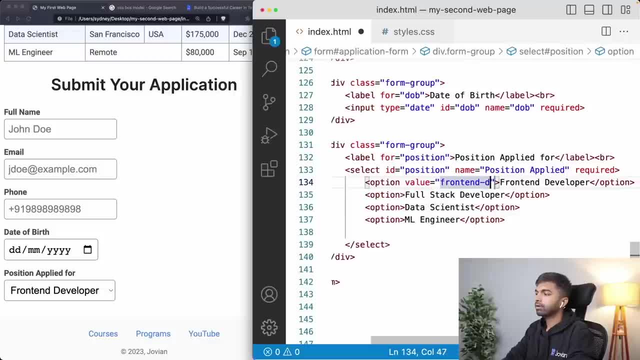 So I'm just going to specify the value- front end, dev or front end here, and I'm going to specify the value- backend or full stack. Okay, Okay, Okay. So this is just to tell you that what you show to the user and what do you actually? 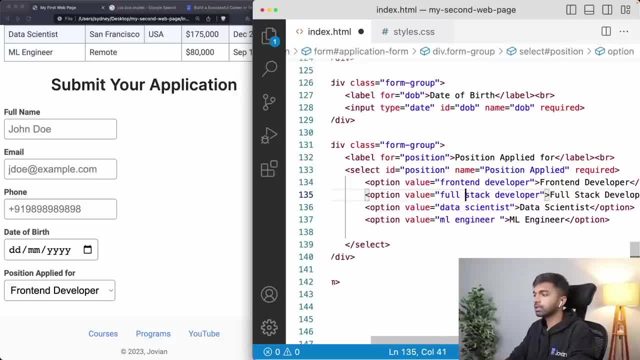 send to the server can be two different things. Okay, When the form is submitted, the server is going to receive this value, But the user is going to see. The user is going to see this value in the dropdown. One last thing that is often done is you have an option with an empty value and that just 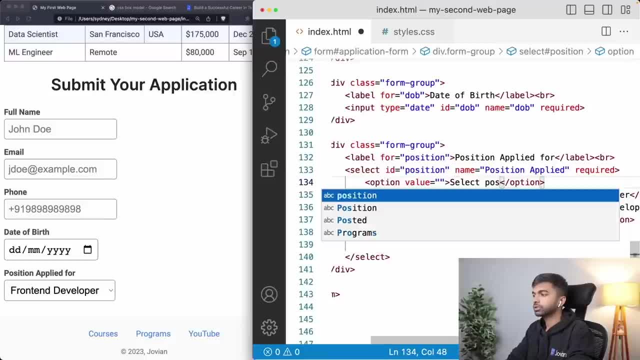 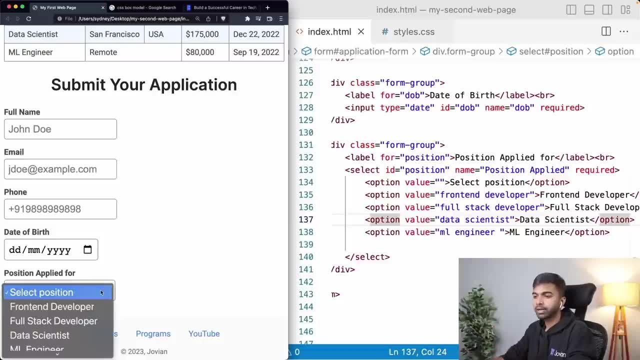 contains an instruction which is select position, right, Something like that. So the idea here is that by default, you don't want to select any position, otherwise that default position can get picked automatically. You want the user to pick a position specifically and that is why you have the select position. 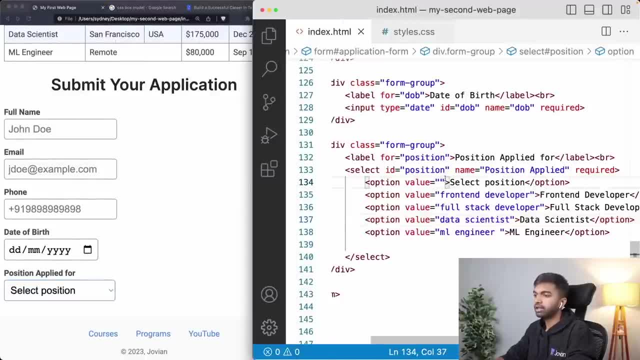 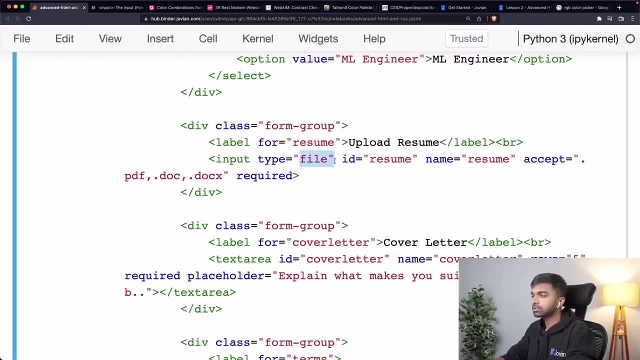 This is like the placeholder option in some sense, And that is often given the empty value: Okay, So that's the value. Then we have file inputs, So file input simply has input. type equals file and we are using file input for resume. 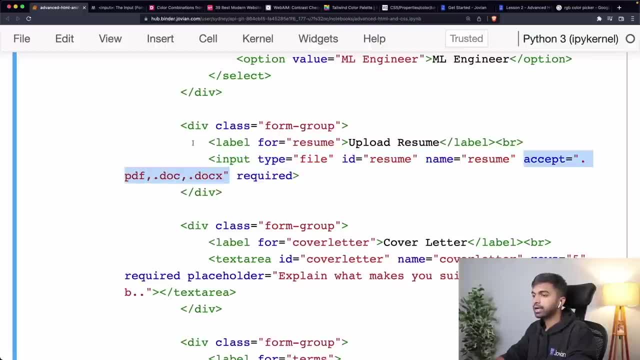 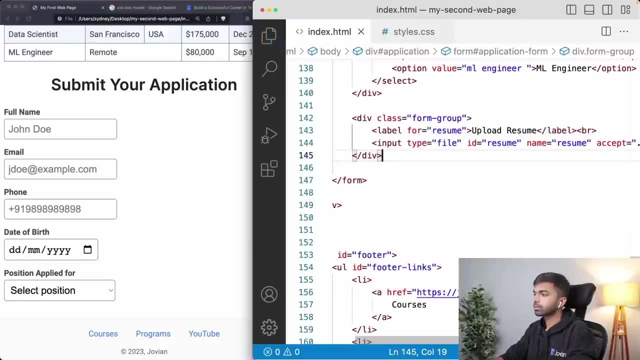 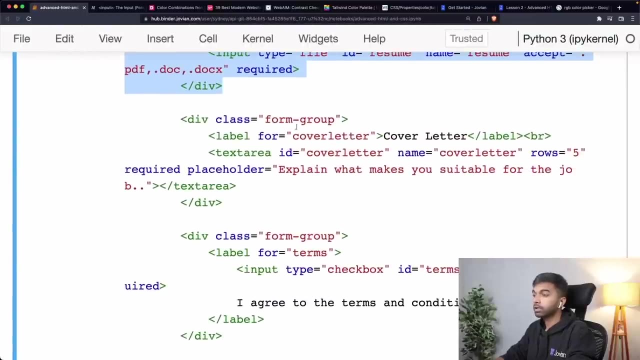 And you can also specify what kinds of files it can accept, like PDF, doc and docx. So let me just come in here, Let me put in the file input here as well. We have this file input. That's great. And then we have this form group for the cover letter. 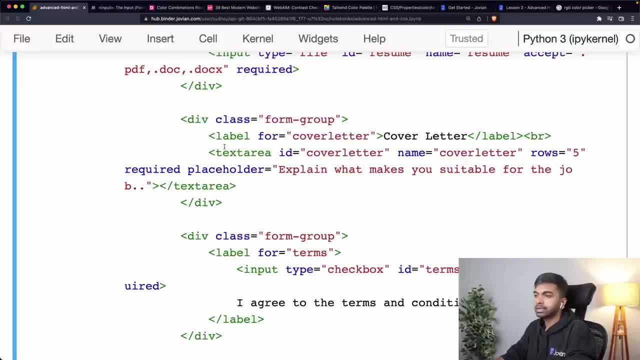 The cover letter. We are using this text area component. So instead of input, we are using text area And again, you specify the ID, you specify a name, You can specify the number of rows that you want in the text area. by default, that can. 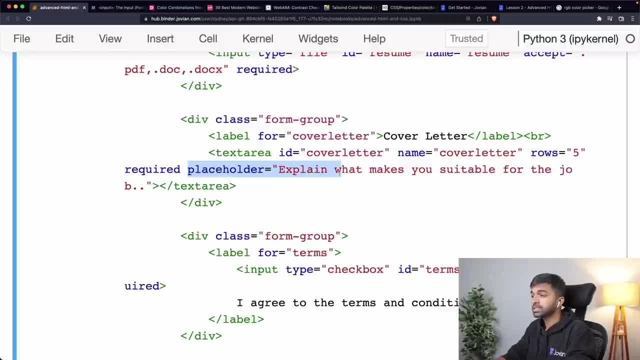 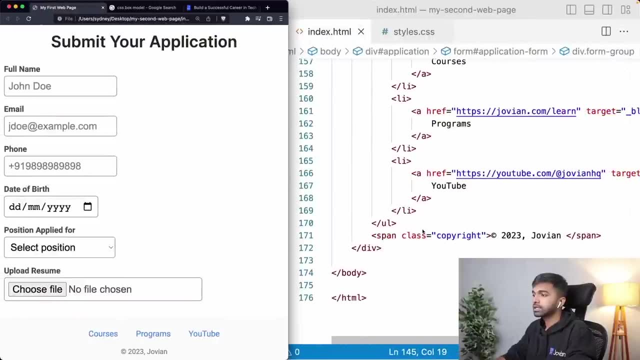 be increased by the user. you can specify whether it's required and you can specify a placeholder as well, but just know that you have to have a closing tag for the text area. Okay, So let's add the text area here as well. 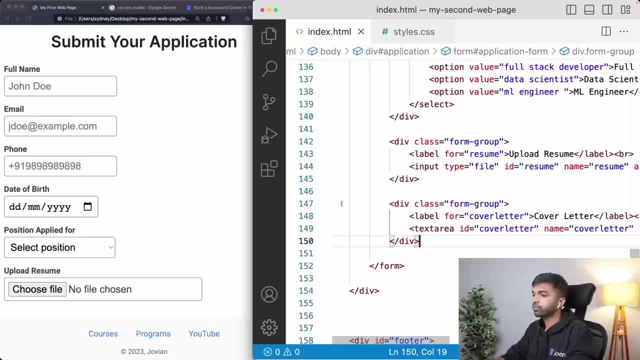 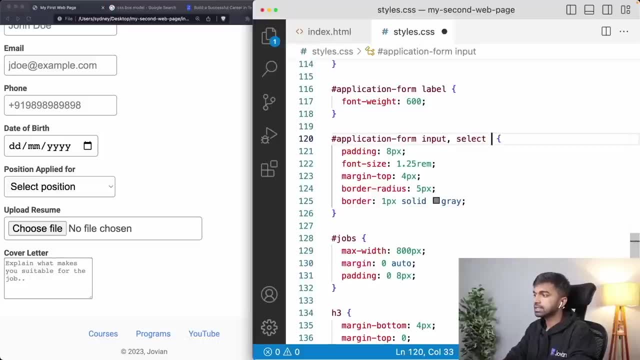 Let us come in here at the text area for the cover letter. Okay, So here we are, asking the user to enter a cover letter as well. Again, I'm going to come in here and I'm going to apply these styles not just to input. 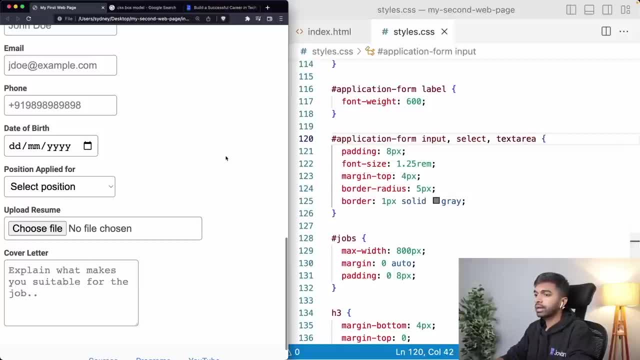 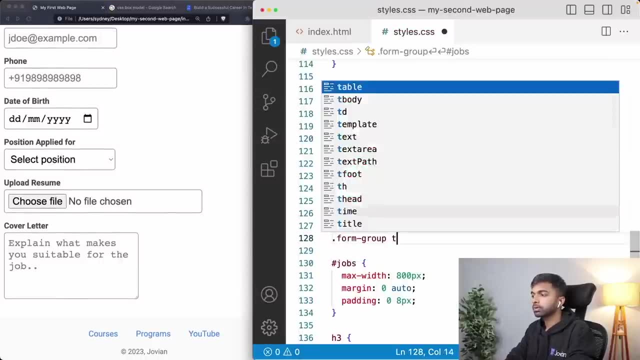 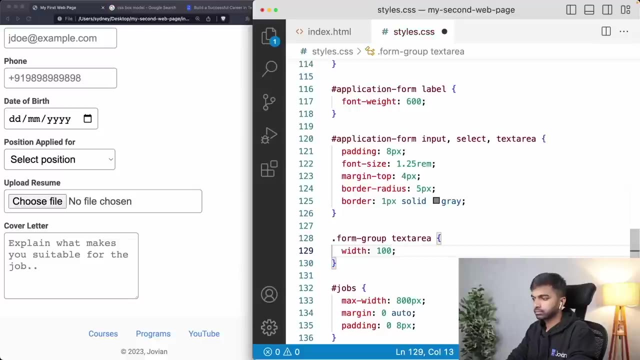 but also to text area, And that way my text area is going to have a better collection. I might want to make the text area full width, So I can say form group, text area width 100%, And this way my text area is going to take up the whole width. 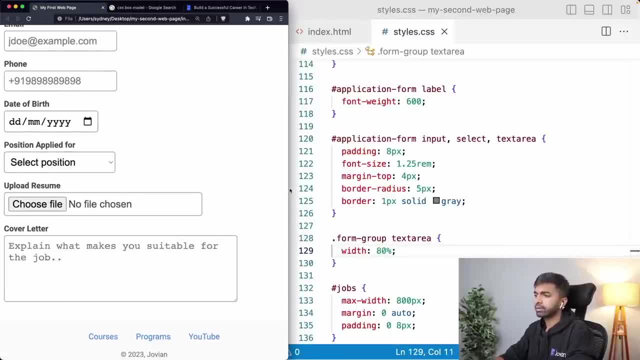 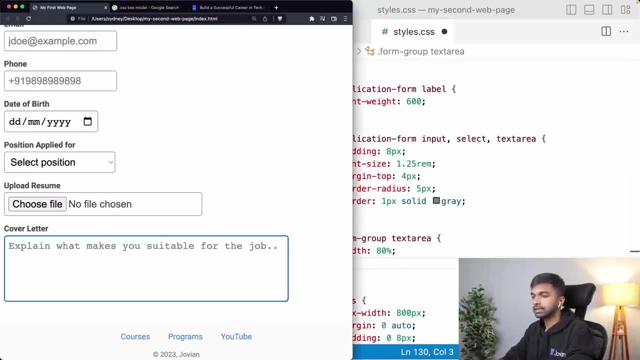 Or at least let me set it to like about 80%. let's say okay. So the text area is slightly bigger and you may also have to specify your fonts or font family for the text area. In this case, clearly it is picking up some random font family. 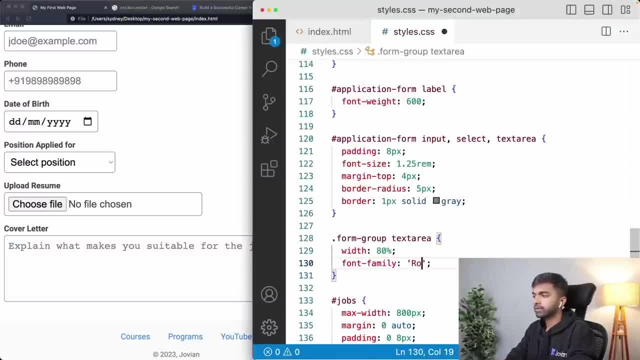 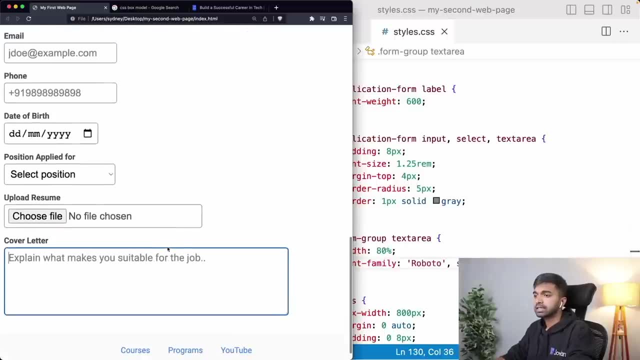 So you also specify font family. Let me specify Roboto, because it is just some normal body text and sans serif. Okay, And now we have specified a text area as well. Okay, Last couple of things. One is a checkbox. So we're going to add a checkbox called iAccess. 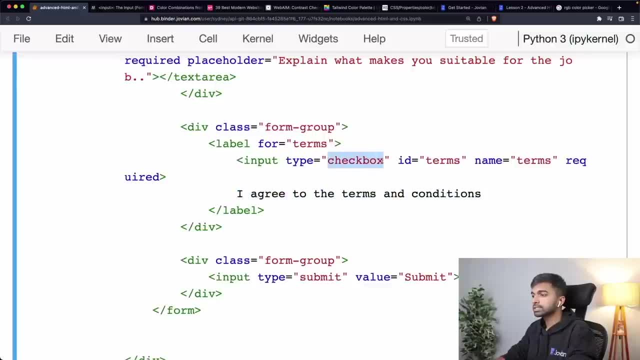 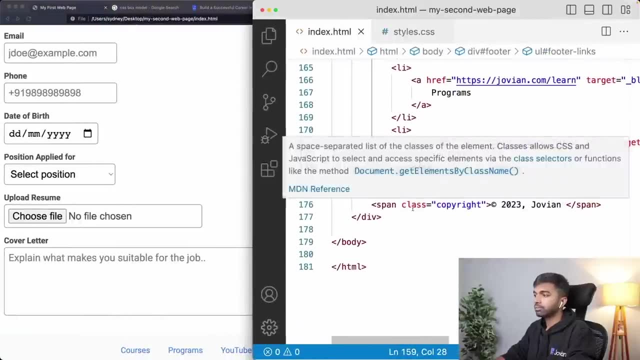 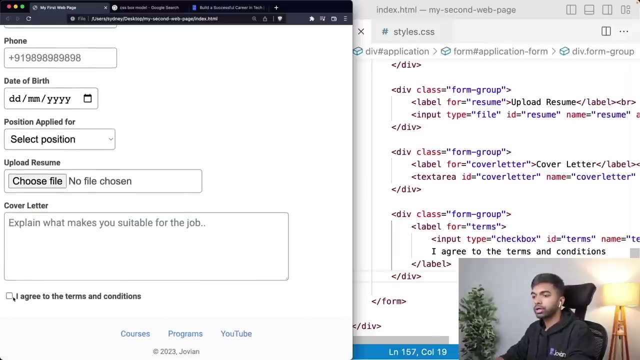 And I agree to the terms and conditions, And all we need to do here is just specify type: checkbox for the input and it's going to show a checkbox. So now, often for a checkbox the checkbox is created slightly differently, Because a checkbox you may require to actually show the input, you may require to show the. 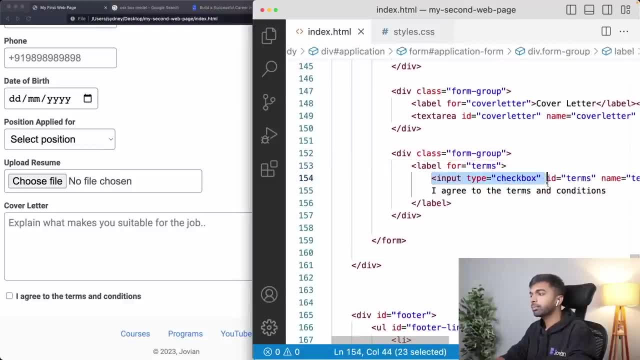 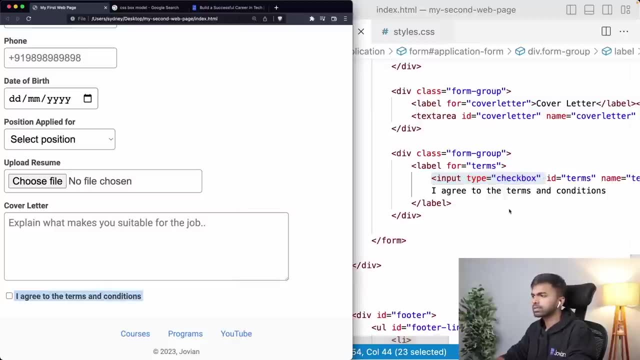 label next to the checkbox. So often in the checkbox what you do is you put the input inside the label And what that does is, if you click on the text as well, that also ticks the checkbox. So that's good. Now, one thing we might want to do is for the input checkbox. I might want to make it. 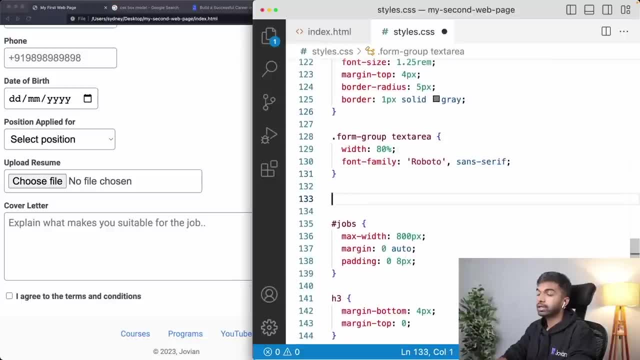 a little bigger So I can do that Again. I'm going to show you another CSS trick here, Not something you need to know right now, But I can say form group input and I can say only for the type checkbox. 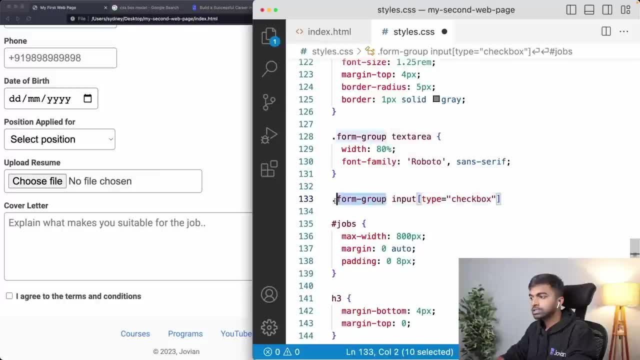 So now I'm selecting in the class form group, I'm selecting an input tag, and I can say only those input tags which have the type attribute set to checkbox Okay, And for them I want to use the width to be 16 pixels and the height also to be 16 pixels. 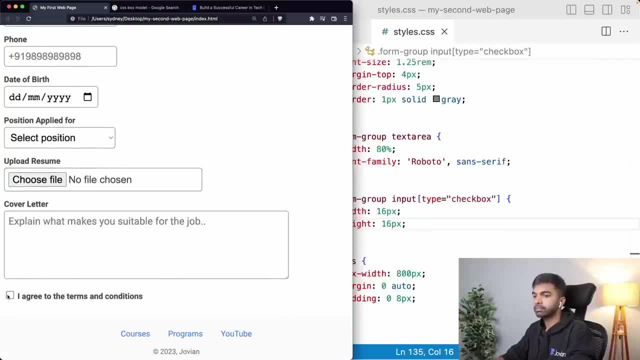 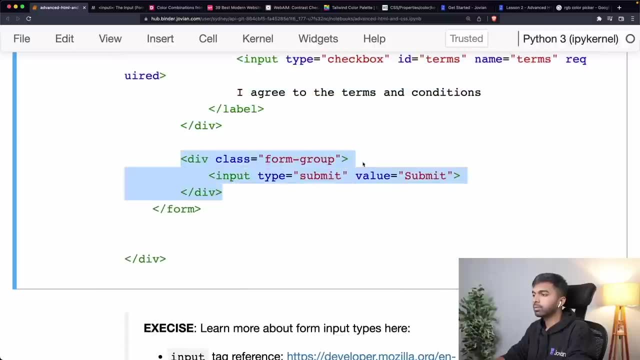 And that is just going to make the checkbox slightly bigger, as you can see here. okay, that makes the checkbox bigger. And finally, we have the submit button. So we just have a div form group input type: submit value equals submit, the value is going. 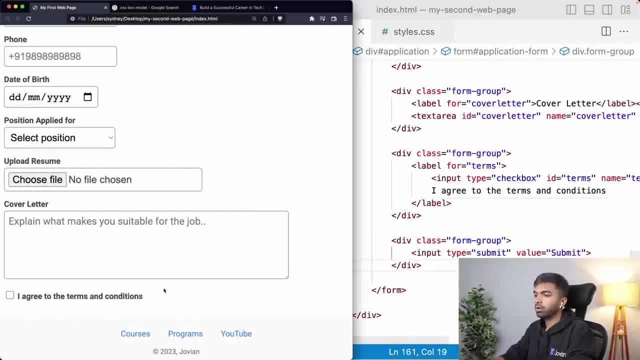 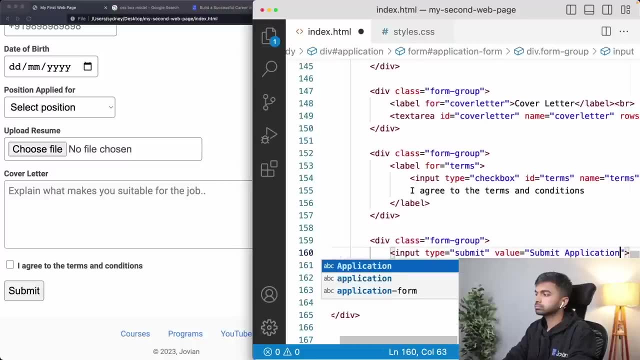 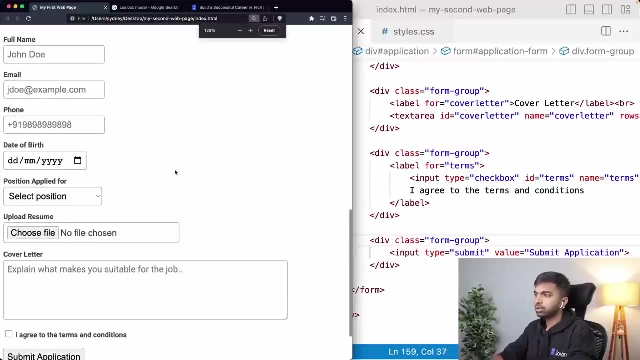 to be whatever you want to show on the actual button. So you could say submit application, Like that, And that is how you create a form. So I'm just going to zoom out a little bit. I'm going to go first, just going to go to 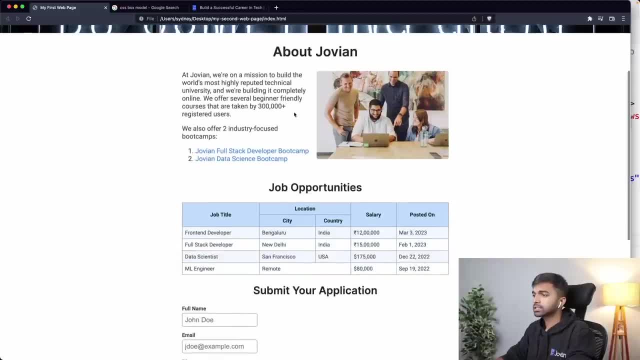 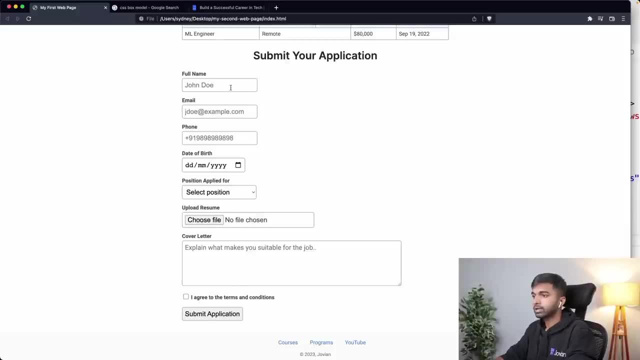 the normal size. So now you have a banner, now you have this description, now you have job opportunities, and then you have submit your application: full name, email, phone, date of birth, etc. And you can fill out all this and then click Submit application. of course, these are all. 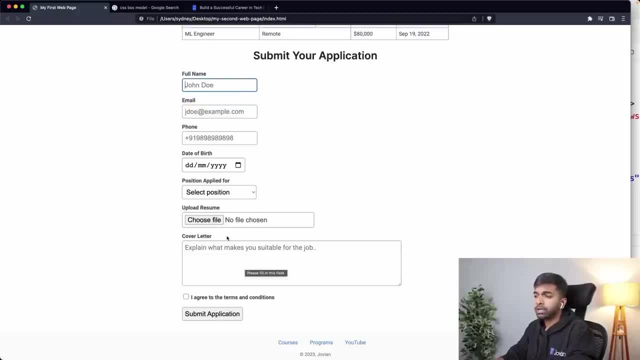 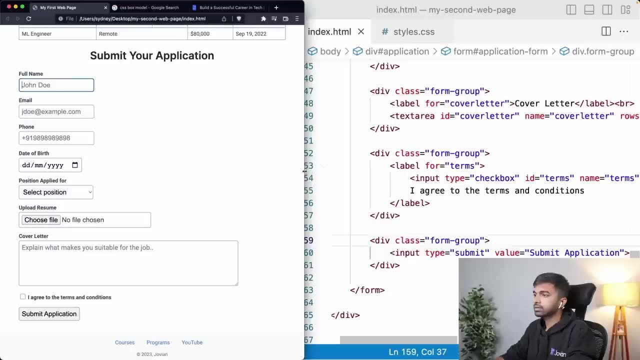 required fields. They will have to be filled in And, if you want, we can make the cover letter optional. So let's do that, so that we can submit without the cover letter for the purpose of testing. Let's bring this back here. 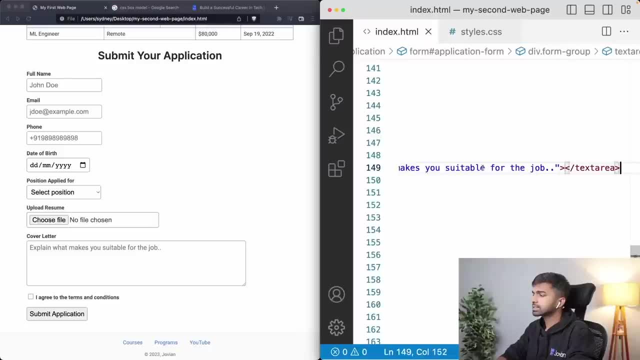 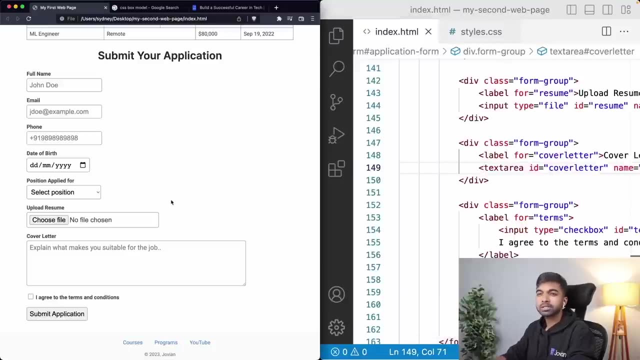 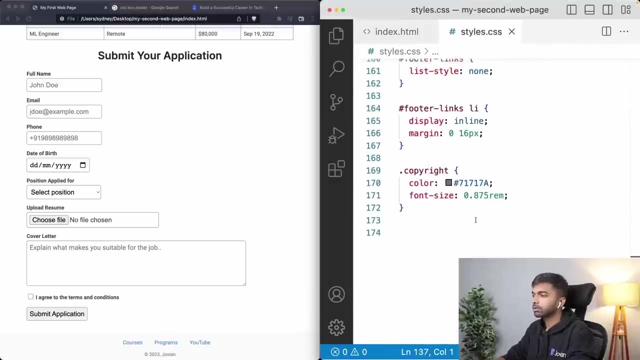 Okay, and let us remove required from here so that this is no longer required. Okay, And now we should be able to submit an application, But let's also add some styles for the submit button. I think a nice blue color would be good to have. 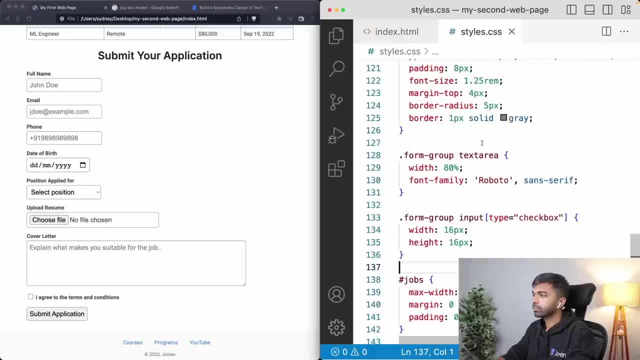 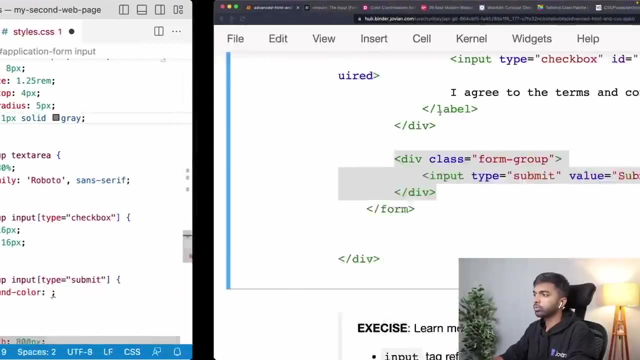 So again I'm going to come in into styles, I am going to select form, group, input type equals submit And I am going to set background color to blue and I'm going to pick a blue from my color scheme. So maybe I'm going to pick blue 500. 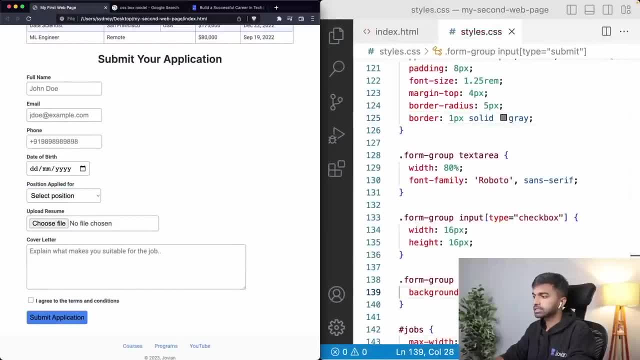 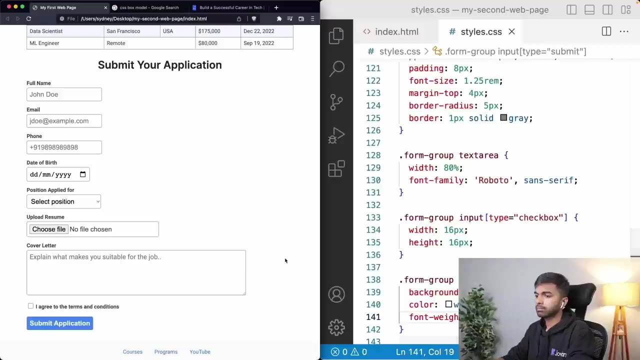 And I'm going to set that as a background color So that looks nice. I may have to make the text Color white. color white. I can make the font weight by less than 600.. The font weight is bigger than maybe 500 might do the job. 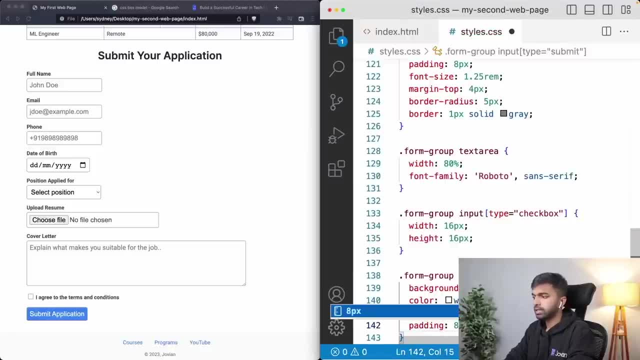 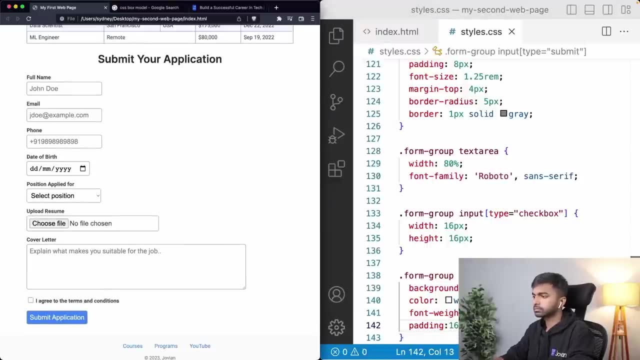 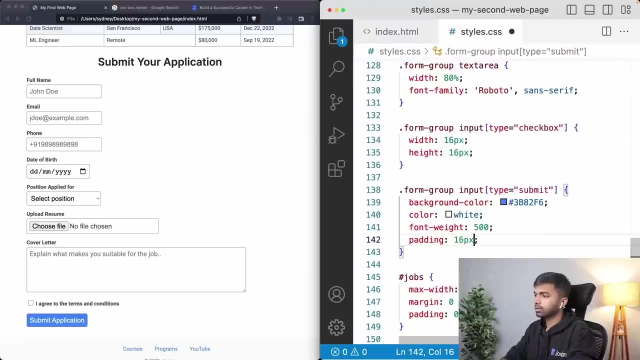 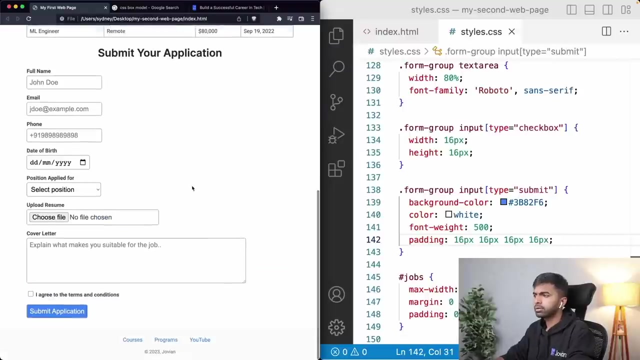 And I can maybe increase the padding 8px, maybe 16px, make it a little bigger, Yeah, Yeah, Okay, So you can specify some things. I think the padding is not getting specified here, but you can specify. it's just a matter. 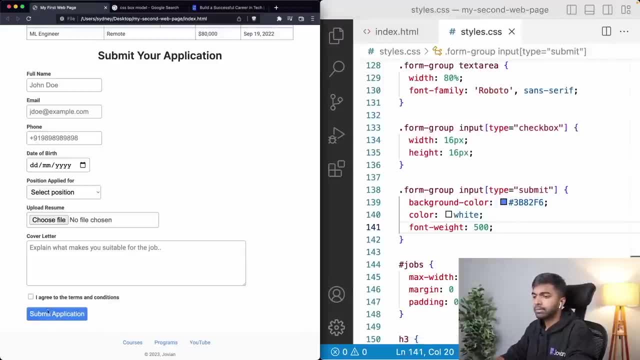 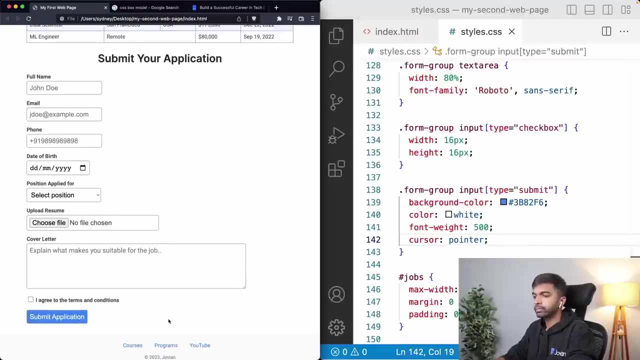 of specificity, I guess, But now my submit application button is actually looking nice. And if I also want, here's another property that you will often use- cursor pointer, And we're going to go ahead and do that. Okay, So what can? what this does is this: converts your cursor into a hand symbol when you have 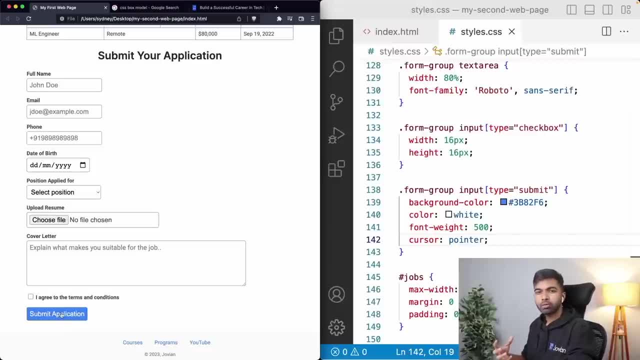 the submit when you hover over the button, and you can also change the hover style. you can change the color of the button when you hover over it, So you can do all sorts of things, And this is something that you should look up and then you should attempt to do. 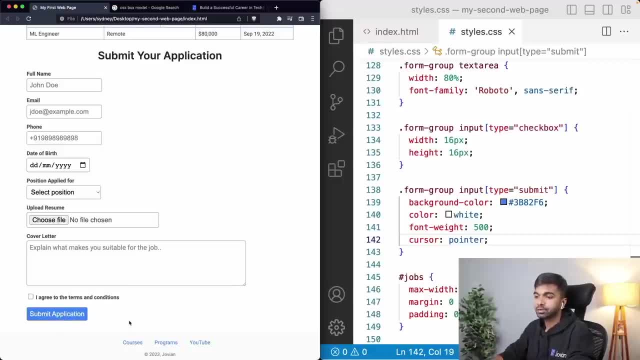 But yeah, at this pay, at this point you click Submit application and that is going to submit the application. So let's try that. So we say Akash a at bcom, Some number. I'm going to pick a date of birth. 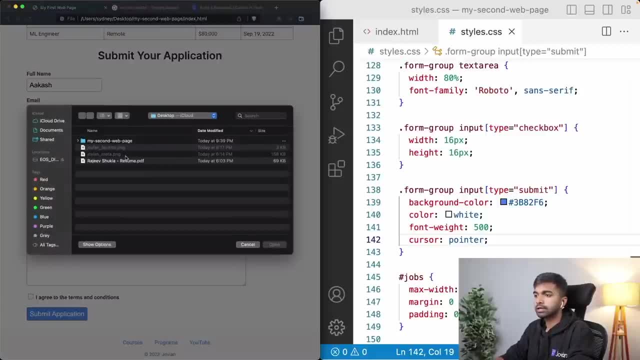 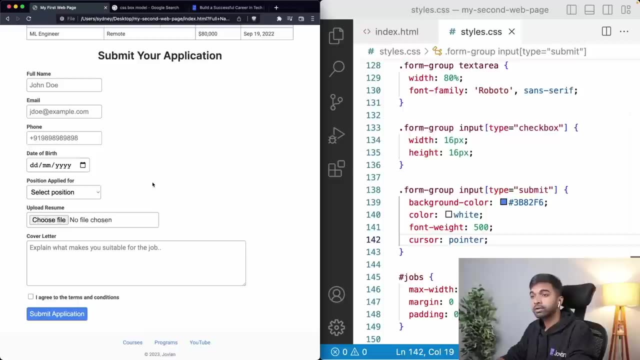 I'm going to select a position. I'm going to select a file, So I have a resume. I'm going to add a cover letter. we're going to submit. okay, it doesn't do anything because we have not configured the form to do anything yet. 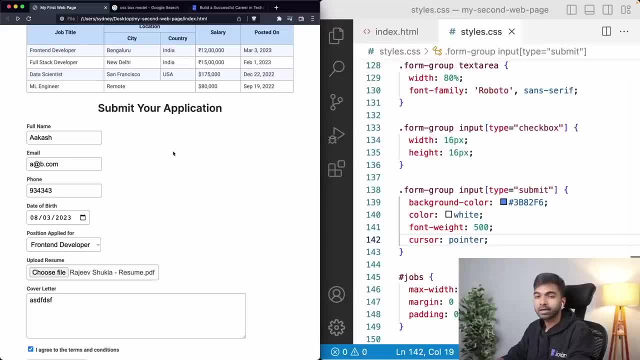 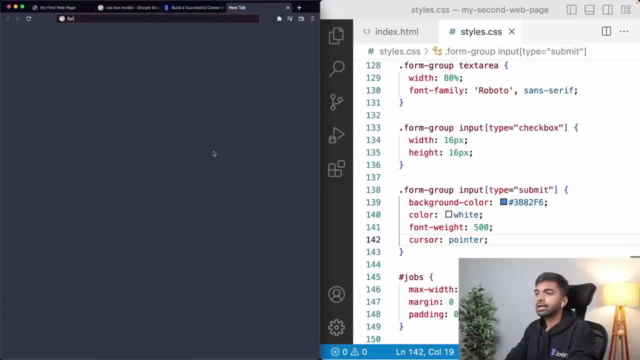 Okay, So what we need to do is we need to send this data somewhere. Normally, this data sent to a server, but we don't have a server right now to process this data. That is where we are going to use an online platform called form bold. 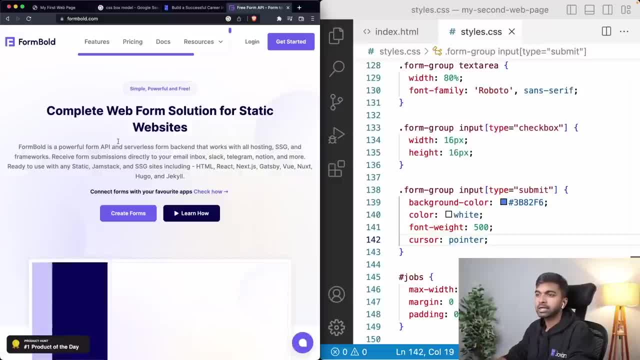 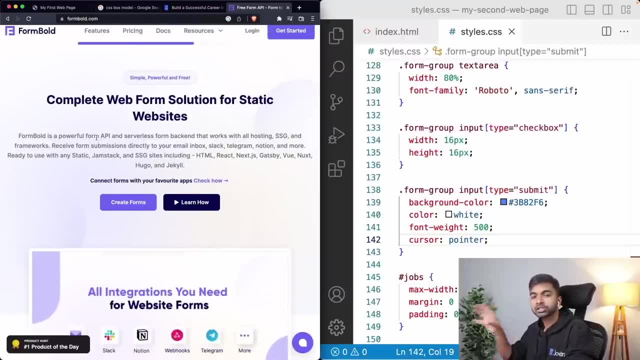 This is not something that you would do in the real world. You can actually. if you're building a personal website, you can use form board. What this does is this allows you to just provide an action for your forms that you are putting into your simple website: static pages. 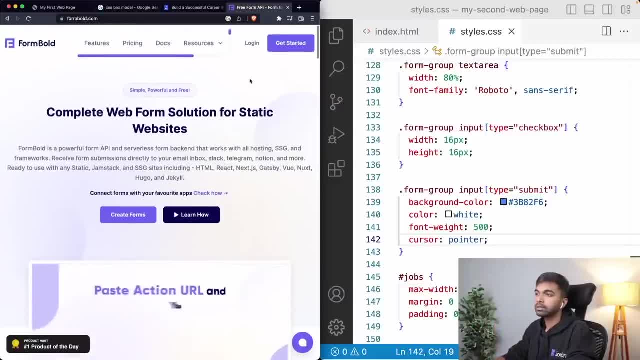 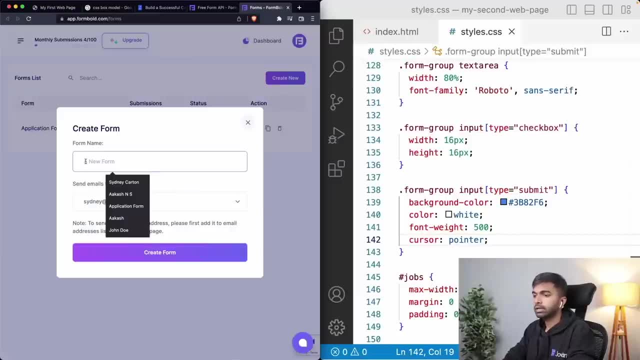 And it is then going to capture those responses and also send it to you over email. So how about I just log in here into form bold and create a new form? Let's call it Jovian application form. Okay, So any new responses that are filled into the form is going are going to be sent to: 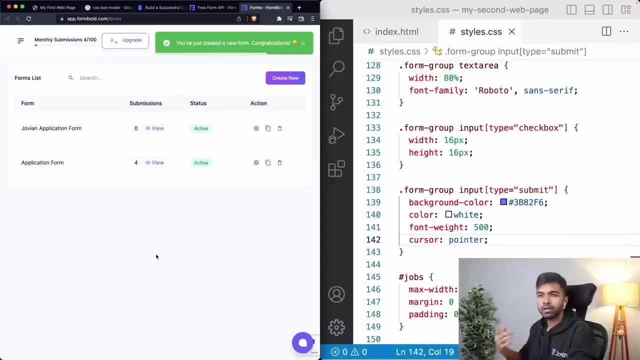 this email And I'm going to create this form. So you may have to verify your email to actually create the form, but I'll let you figure that out. Okay, and now let's open this form. So let's go into the form settings. 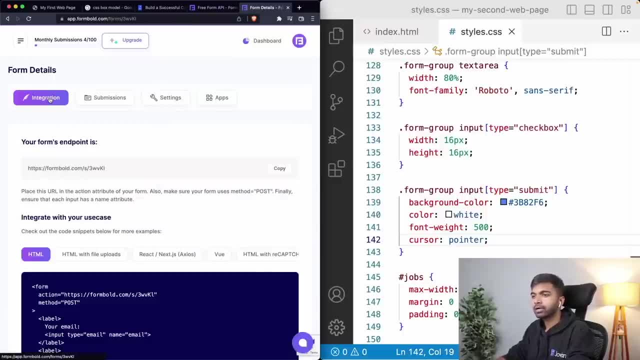 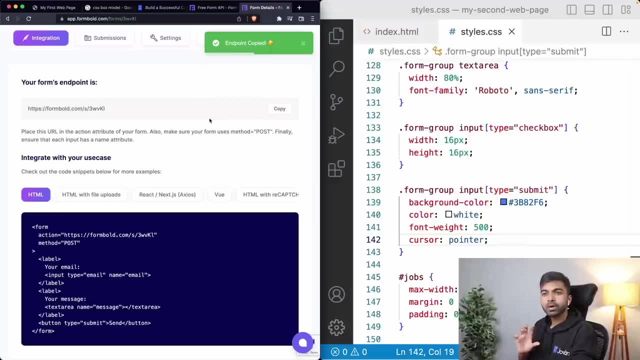 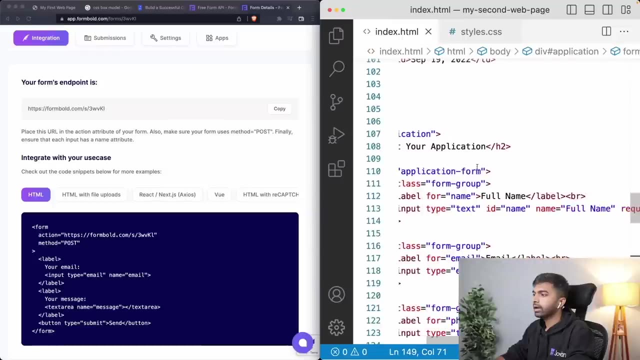 And in the form settings you will see this integration option. So let's click on integration And here it's going to give this endpoint, So just copy this endpoint. Okay, This is where we want to send our form data, So copy that and come back here into the form. 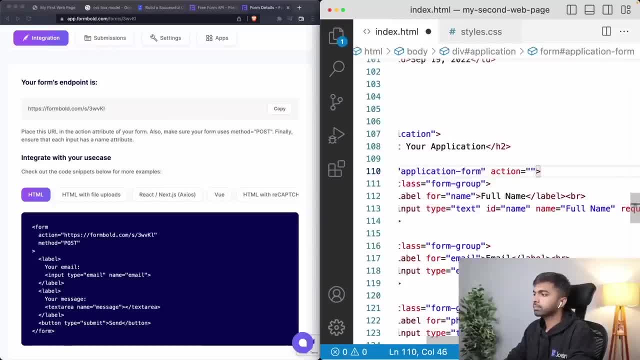 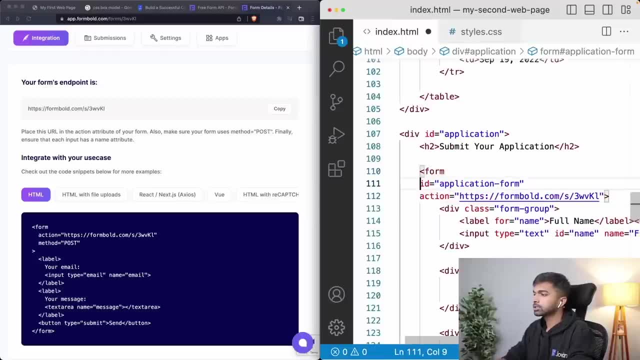 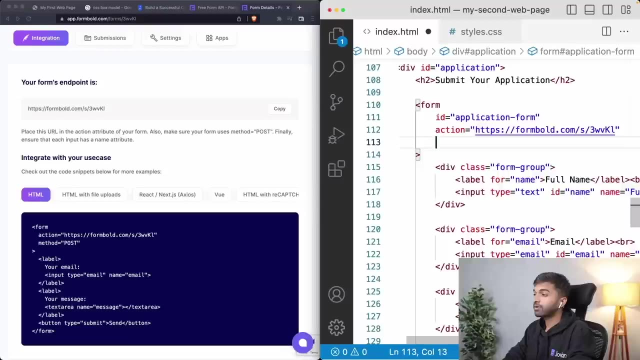 And what we can do is we can say: action equals this link. I'm just going to put it all here so that you can see clearly: Action equals this link, Okay. And we also have to specify a method And you can see how, you can see an example of how it, how this form should be used. 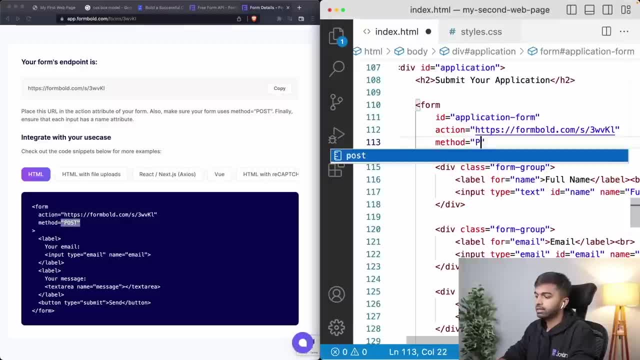 So action is this: link And method is post. the method equals post And let's just save that. And since we want an HTML form with a file upload, I'm just going to select this option with a file upload. So I think we also need to put in this ink type multi part form data. 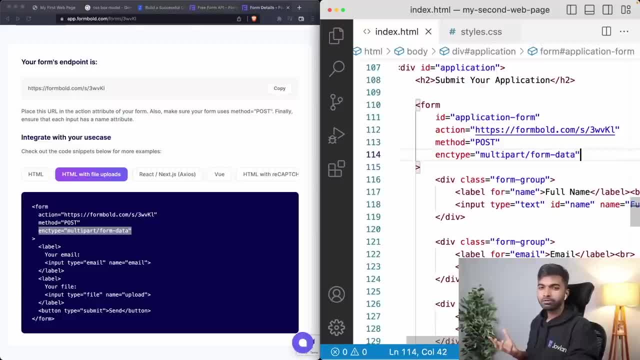 Okay, Don't worry too much about what these mean. Whenever you're using a form, you will have to set these. sometimes these will be set by your own server, So we are going to look to revisit forms in a lot of retail later. 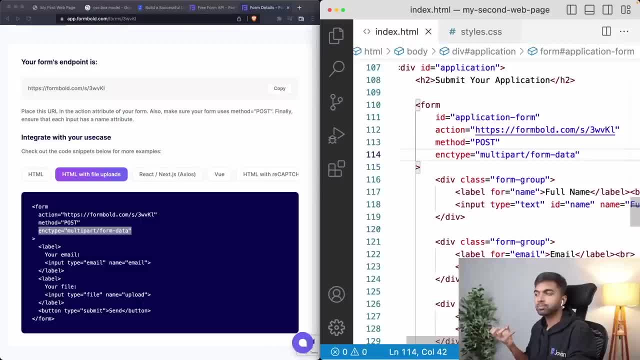 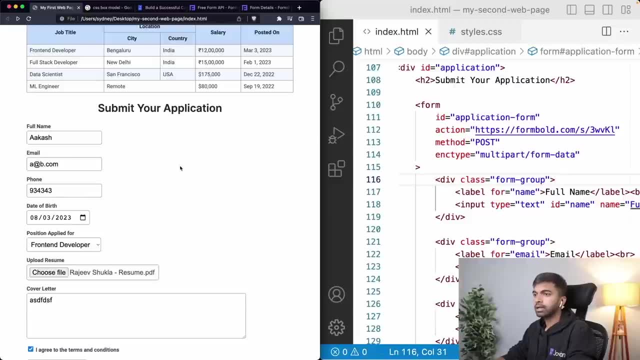 But for now we're just using a third party service. Okay, We're going to capture these form responses for us when we hit the submit button. Okay, Let me save that, And now I can come back here and I can reload the page and I can start filling something. 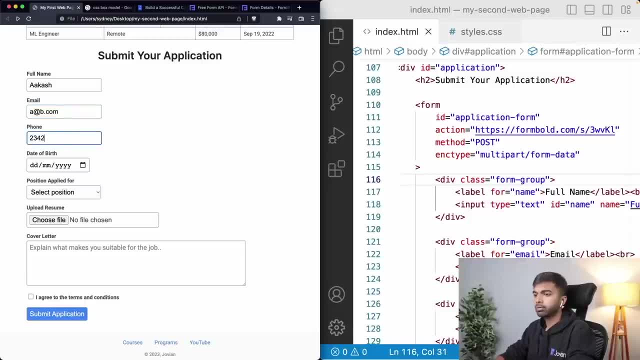 So Akash a at bcom and put in a number, put in a date here, put in a full stack developer, choose a file and put in some cover letter here, agree to the terms and conditions and click submit. Now, when we click submit, it is going to send all the data. 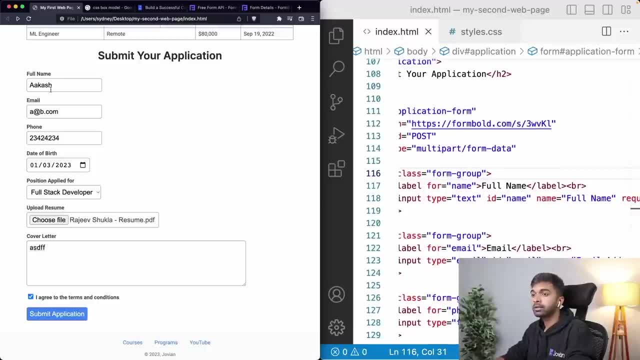 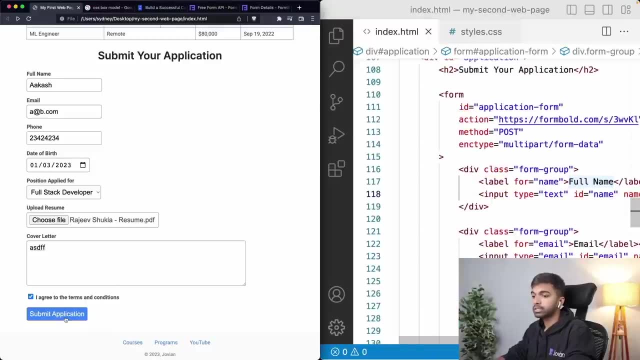 Okay, So this is going to be as those. each or each piece of data picked up is going to be associated with the name property that we have specified, the name attribute, and it is going to be sent into the form. Okay, So I click submit application and you can see that it has sent the data to this form. 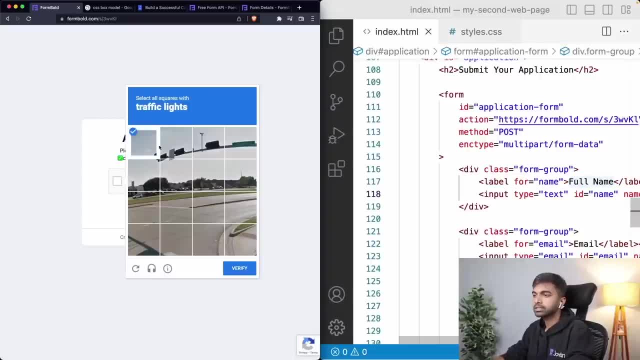 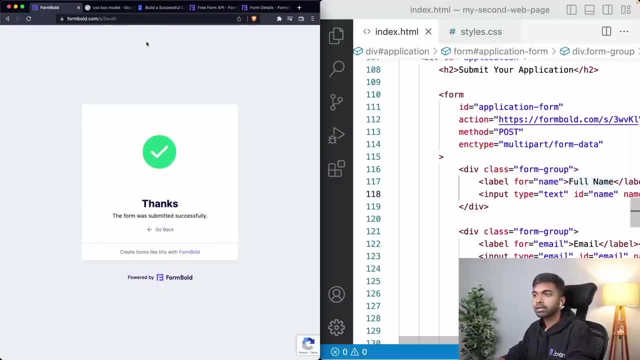 and this form board. the service that we're using is asking us to maybe just verify traffic lights to prevent spam, And once it checks that the form is submitted, Okay, Now I can come back here on the form board page And I can go into the submissions. 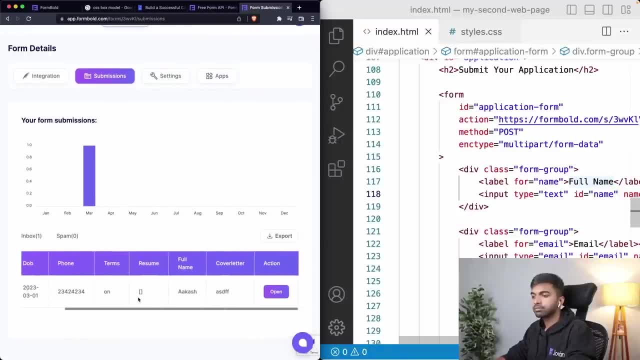 You can see that one submission was obtained and these were the values that were filled in full name: Akash. cover letter: empty and the file is not showing up because there's a way to view files, maybe in some other way, but they've accepted the term. 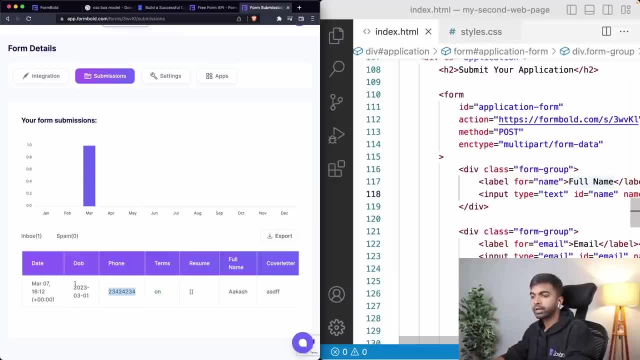 So if a checkbox is ticked, it is marked as on, and then the form and then the date of birth. all of it is present And the data at which this form response was created was also captured by form form board, but that is something that you can pick. 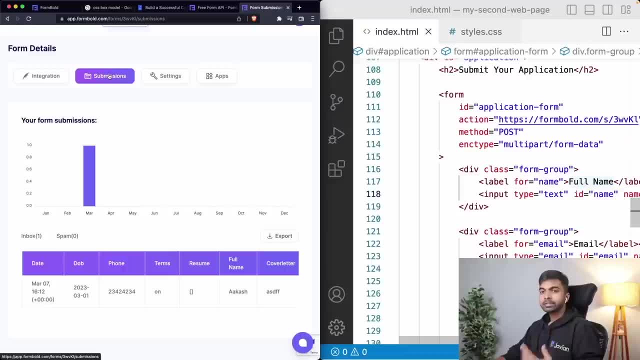 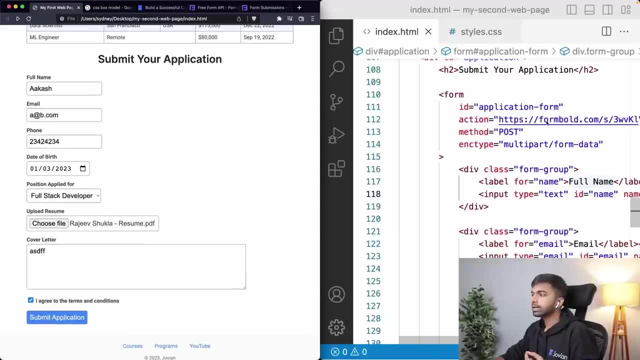 Okay, On your own server, Okay. So the idea is not to tell you that you have to use form bold for all your forms. The idea is to tell you that every form requires an action to be specified and a method or method, and action is something we'll talk about in a lot of detail later. 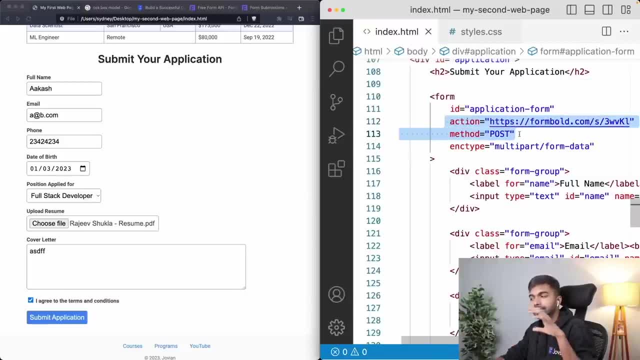 So don't get confused right now, but the form data when is collected and sent to the server, which processes it in whatever way it wants. it can process it and send an email. It can process it and maybe make a database entry. All right, 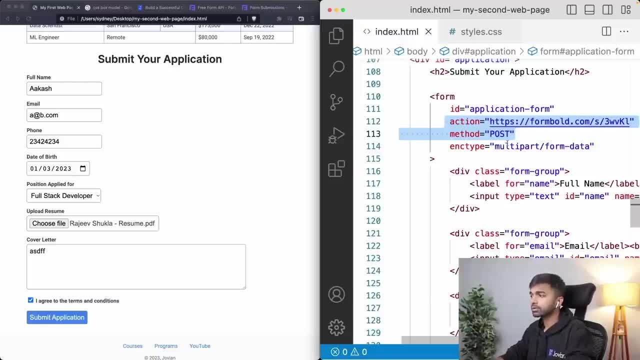 I'll show it and just show you on the screen, like that. However, it is Okay, But this is how you create HTML forms: by creating these um, by picking these tags and by using the input and the label tags and then styling them as required. 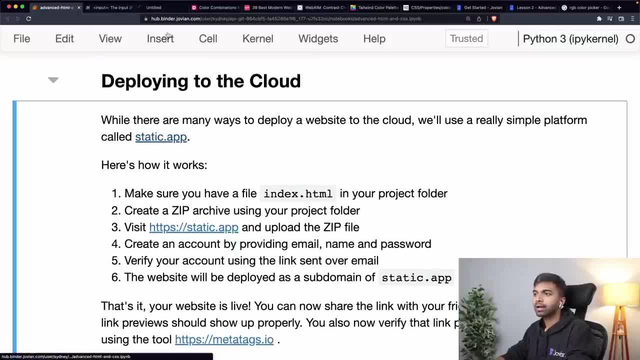 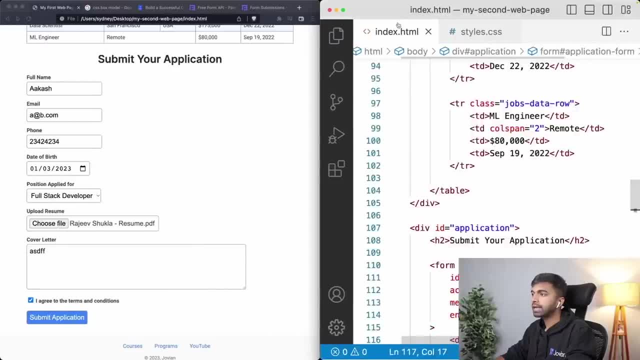 So, to deploy this webpage once again, we can go to staticapp And it is a simple application, that a simple web application that can be used to simply upload a zip file. I'm going to come back here. I am going to simply zip up this folder. 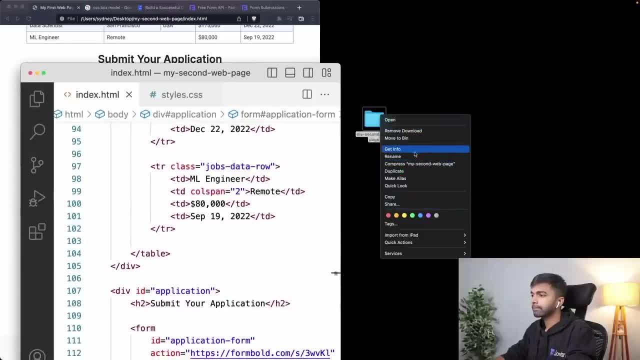 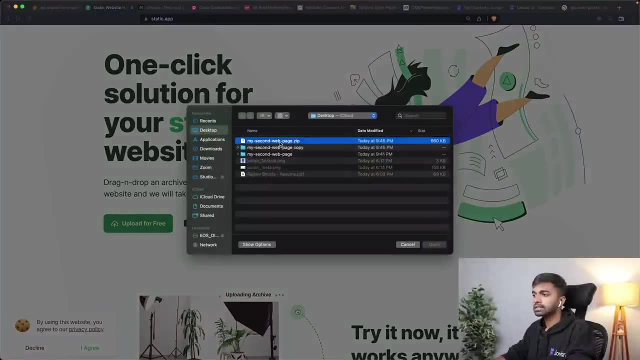 My second webpage. Let me just zip it and press. This was a copy, Let me. let me create a zip file. compress. zip file has been created. Now I'm going to upload it. I'm going to select the zip file and I am going to just pick whatever domain name it's. 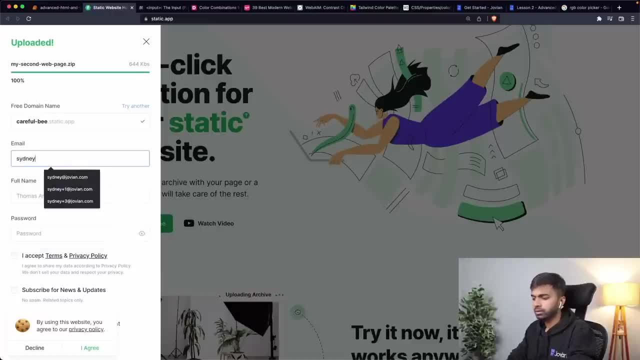 giving me I'm going to put in my email. so I'm just creating a new account here. So that's where I am putting in this plus 10 to create a new account. Um, Sydney Jovian, let me create a password. 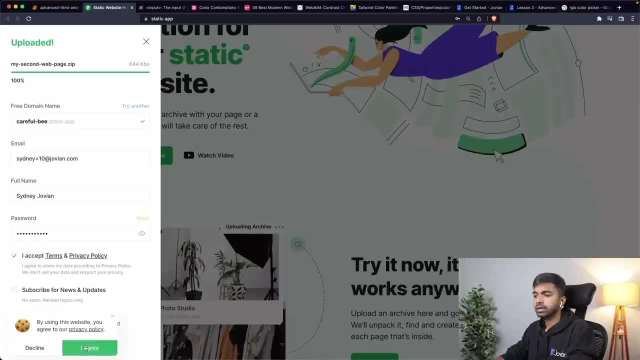 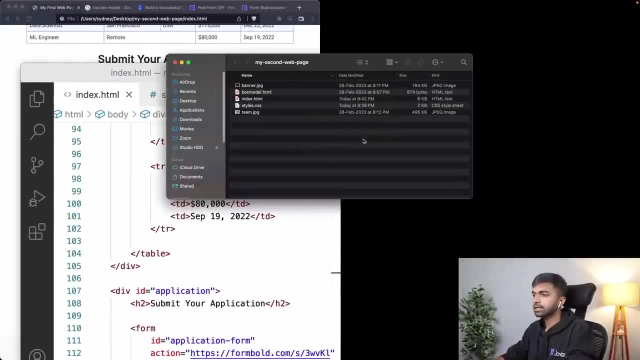 Let me accept the terms and let's continue. And it should ask it should upload the CSS file. So of course this contains our index or HTML. It also contains a team and the banner files and it contains maybe a couple of other styles. 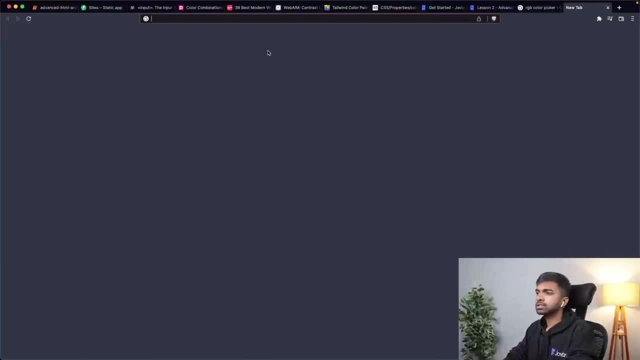 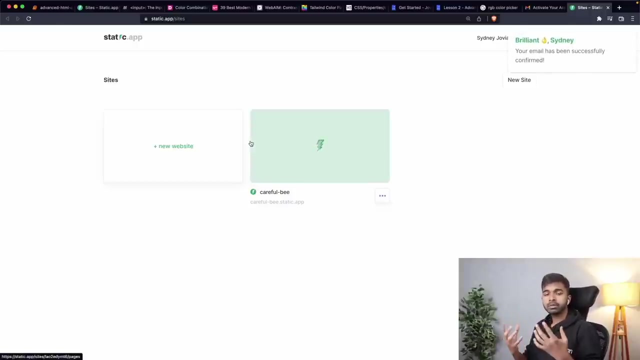 for CSS file. Okay, Okay. So I'm just going to go in into email and verify my email. Let's verify my email address. And now what we have done is we have taken the code that we have written, which contained the HTML file, the CSS file and a couple of images. 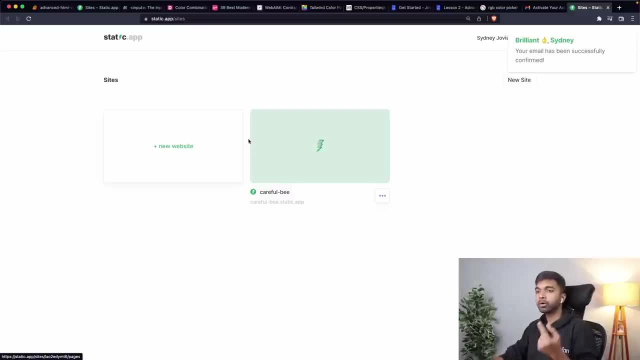 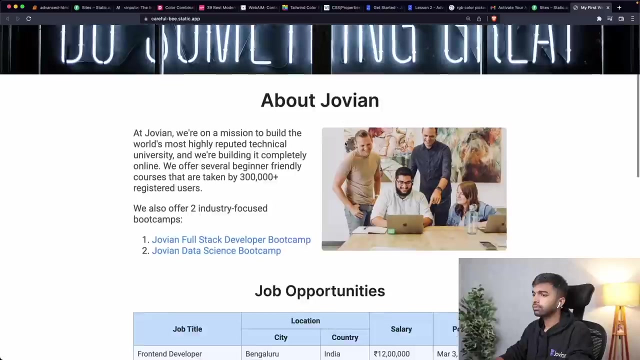 We've put that in a CSS or put that in a zip file and we've uploaded that zip file to staticapp and that zip file should now get deployed as a website at careful B dot staticapp. We have the website deployed. We have this header over here. do something great. 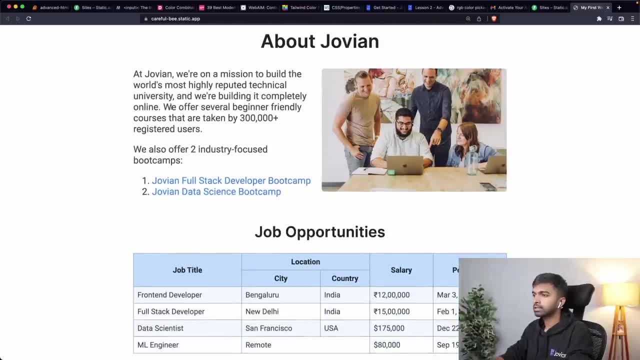 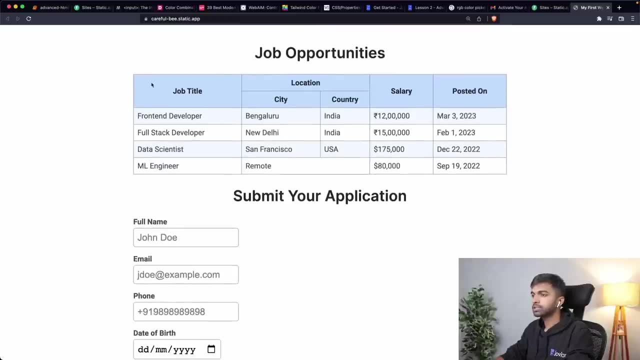 We have some information about Jovian. Now it is using the colors and the fonts that we want. on Jovian, We have these nice links that are colored using our theme, our primary color. We have these job opportunities over here, and then we have a place to create and submit. 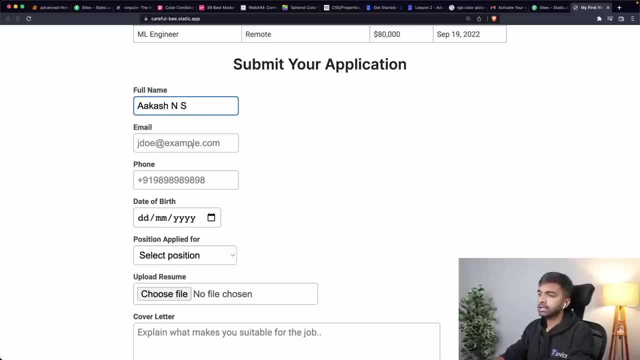 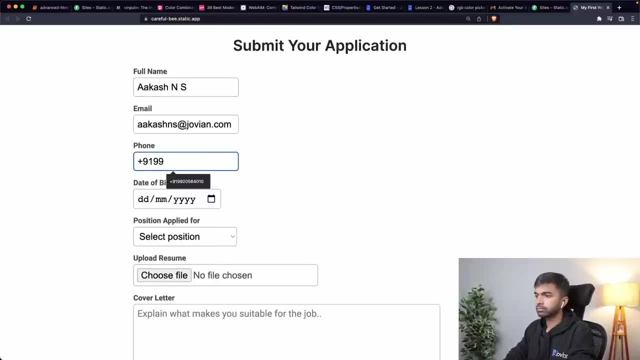 an application And I can go in here and I can say Akash NS, I can say akashnsjoviancom, I can put in my phone number And I can select my date of birth. go back, select a date of birth from long ago. 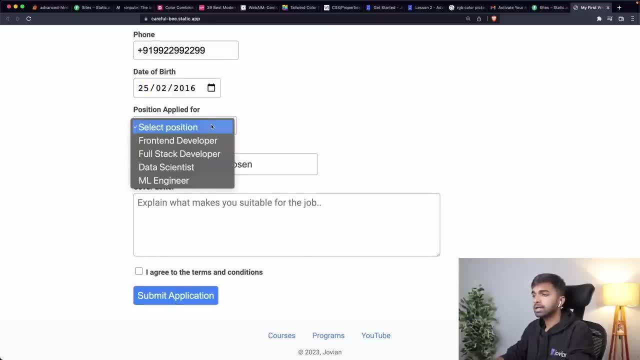 And if I try to submit without filling everything, I'll have to fill it. I can select a position, Let's say full stack developer. I can upload a resume. I can pick a cover letter. This is a cover letter. I agree to the terms and conditions and I click submit application. 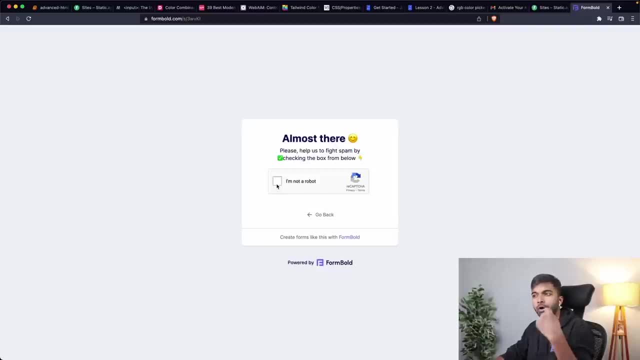 Okay, And that Pushes the data to form tape form board. That is the third party online service we are using for our website- is on staticapp and it is sending data to form bold because staticapp cannot run a server. It can simply show your pages as they are. 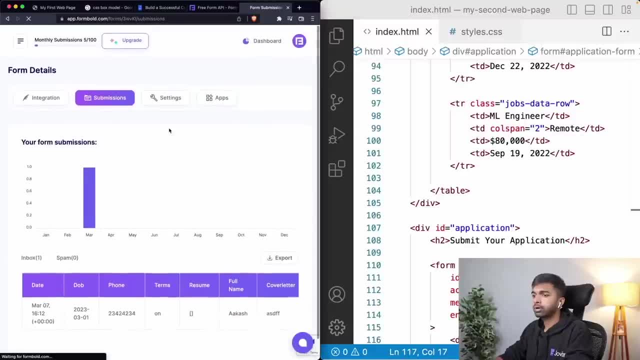 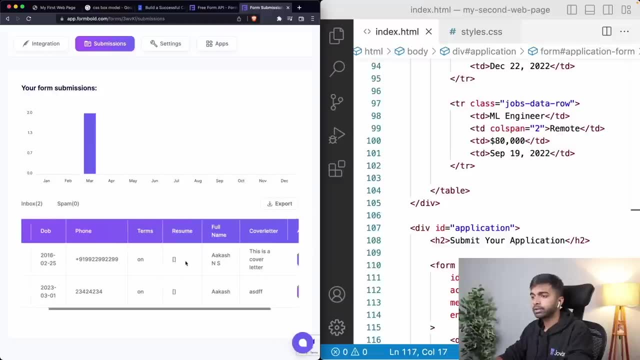 Okay, And once that is submitted, I should be able to check in on my form board dashboard that there is a second application by me. This is a cover letter, This is the phone, date of birth terms accepted, et cetera. Okay, 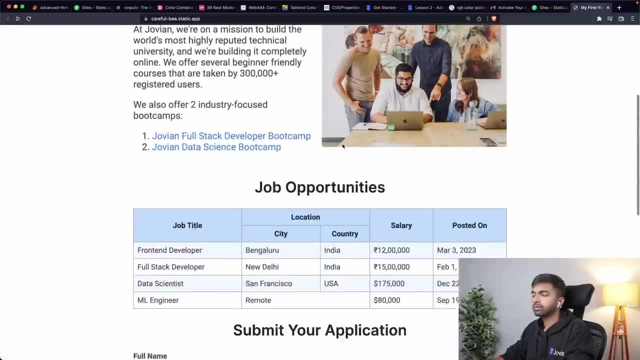 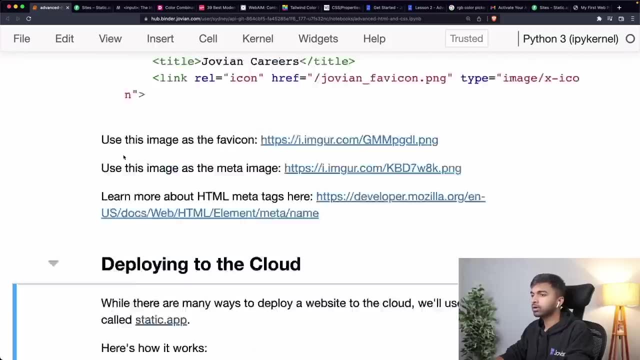 You can also see it in more detail over here, and now we can go back and we can fill out the form again. Okay, So, yep, you can try this out. And there is one last topic which we have not gotten to today, which is adding meta. 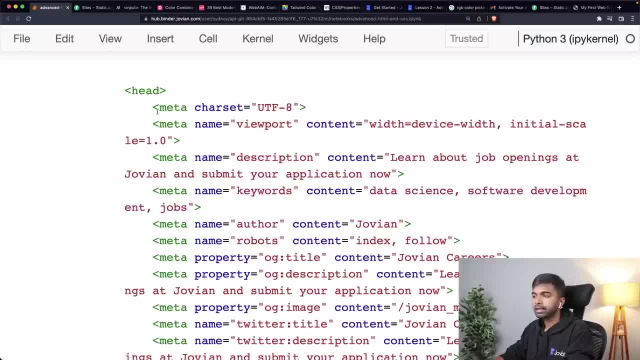 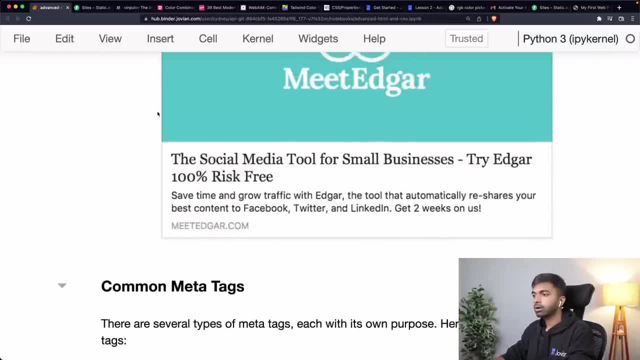 tags. So there are a bunch of these tags that go in the head tag And what they do is they determine what shows up when you share that page online, or let's say, when you share that page on Facebook. what is this preview image that should show? 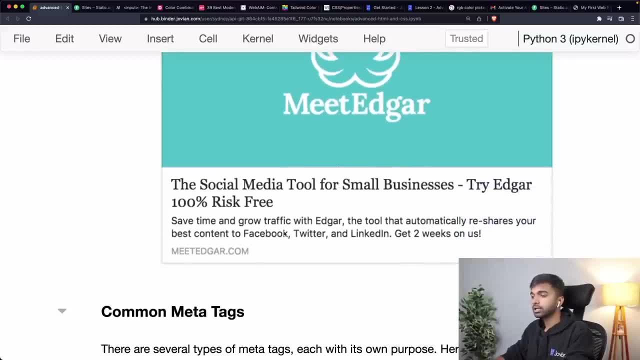 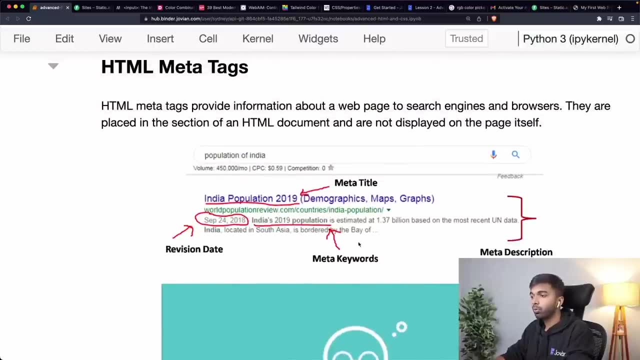 up. What is the page title that should show up? What is the page description that should show up? That is something that you can actually configure within HTML. Similarly, when Google finds your page, what is the information it sees and it displays in a search result? 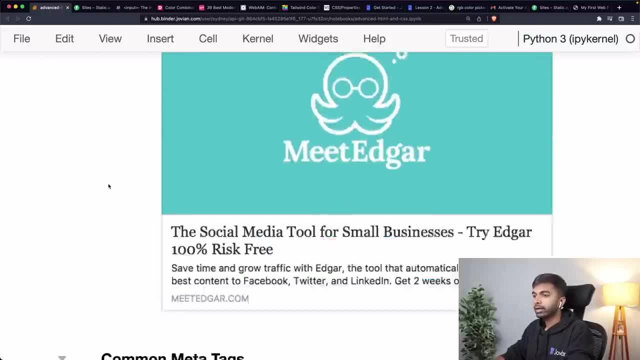 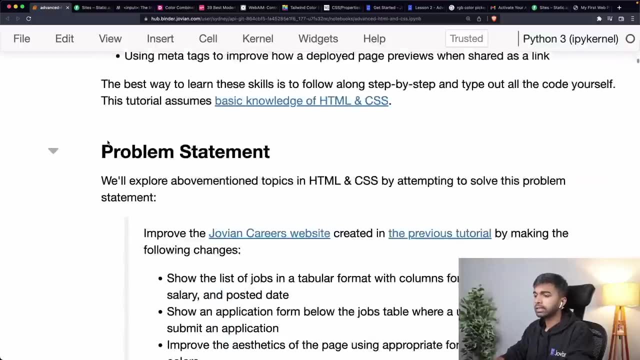 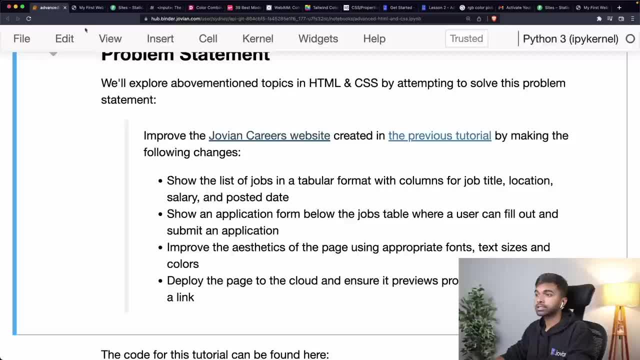 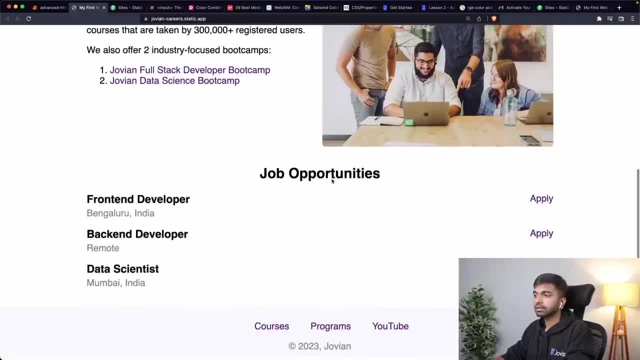 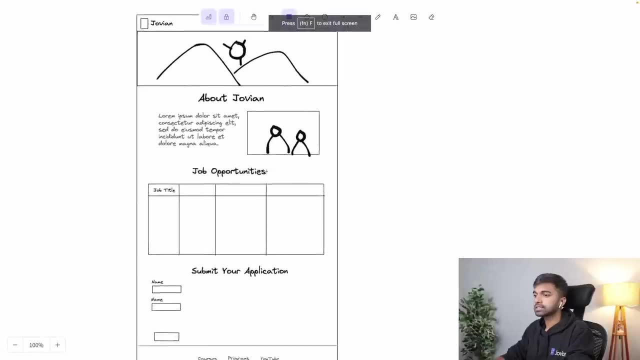 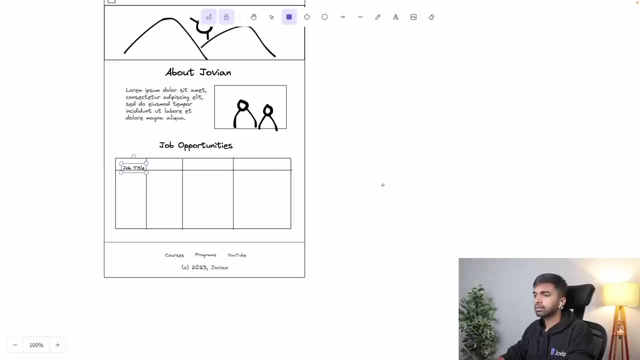 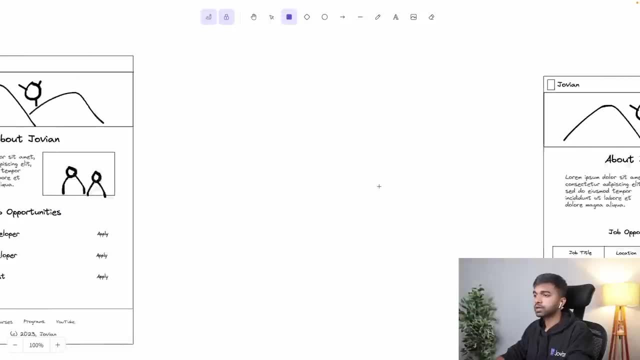 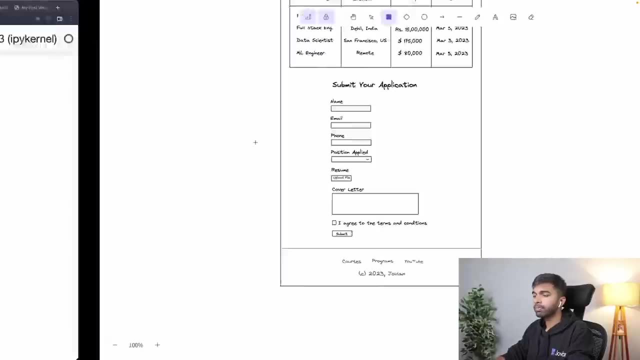 this initial wireframe which looked like that. We wanted to improve this wireframe, So we made it look like this. but we have this table and we have the submit, your application form, So that gave us a visual reference for what we wanted to create. 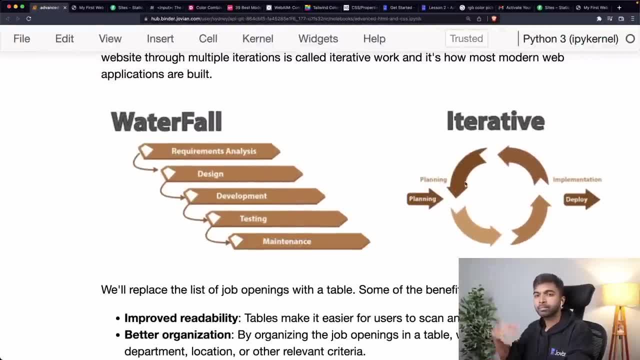 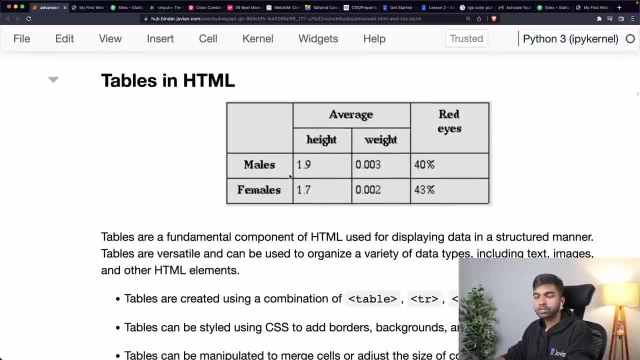 And of course this is the iterative method of software development. You build something, deploy it and let people use it. Then you come back. I can improve it. And then we came in and we created a table. So we created tables using the T table, TR and TD tags and also the TH tags. 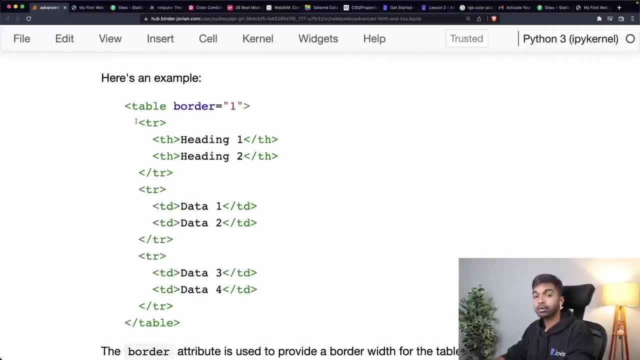 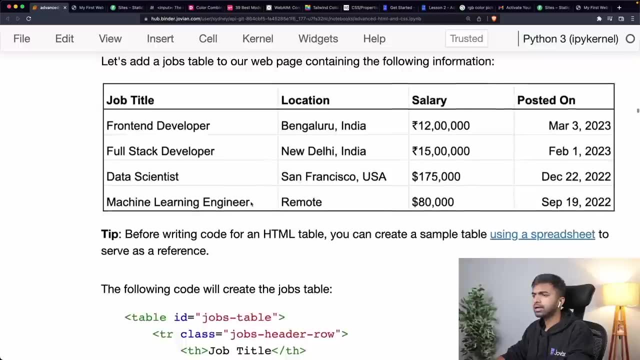 So you first create a table tag, You then create the rows using the TR tag, Then you create heading cells using TH and data cells using TD. And we just did that. We looked at some data that we had put onto a spreadsheet and we just transferred that. 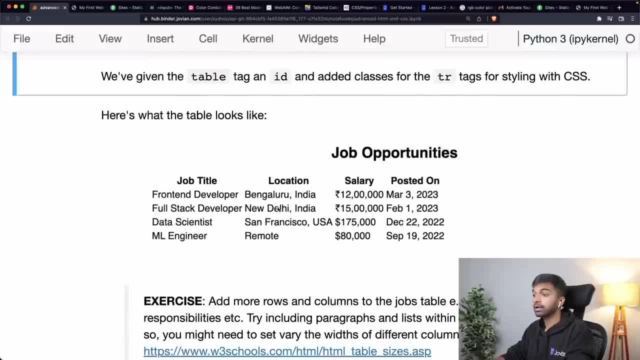 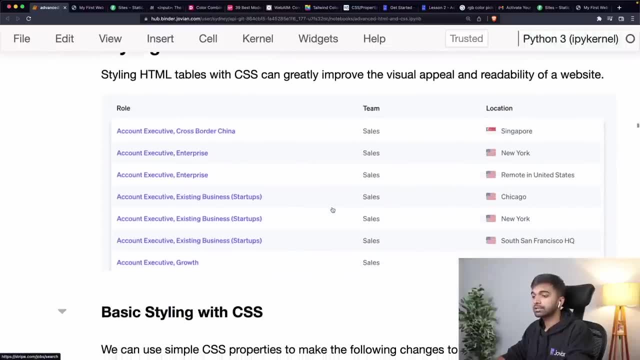 into HTML code And that allowed us to create a table That looked like this. Of course, we this is not a very pretty looking table, So the next step was to style the HTML table to make it look a little nicer, And the basic styling that we did with CSS was adding borders around the table and the 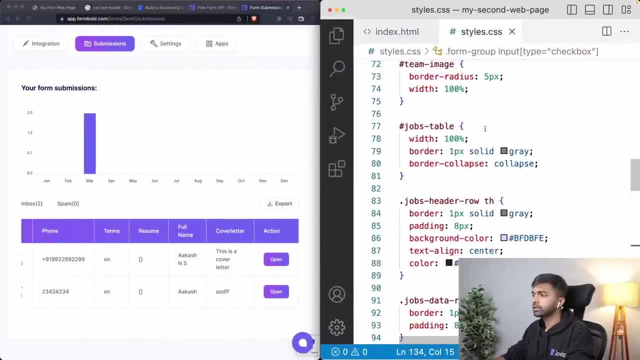 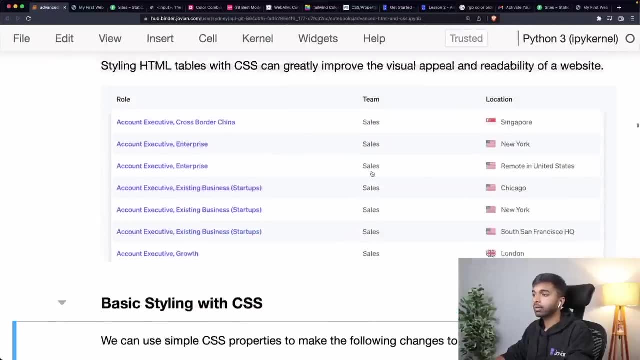 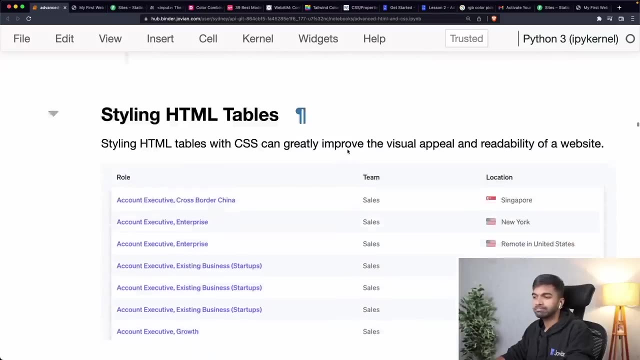 table cells. So you can see, here we've added borders, or the jobs table. Also we've said border collapse equal to collapse, Otherwise we get these double borders that we were looking at earlier. So to avoid the double borders like this, you have to set the border collapse property. 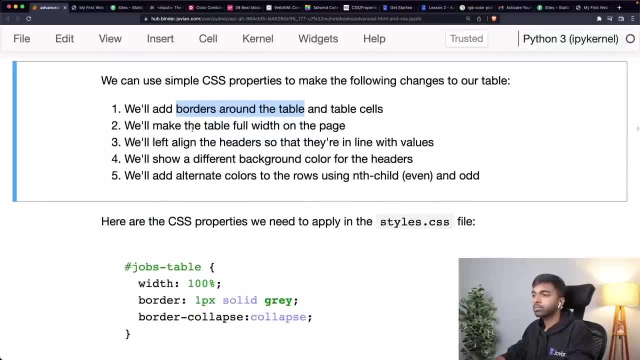 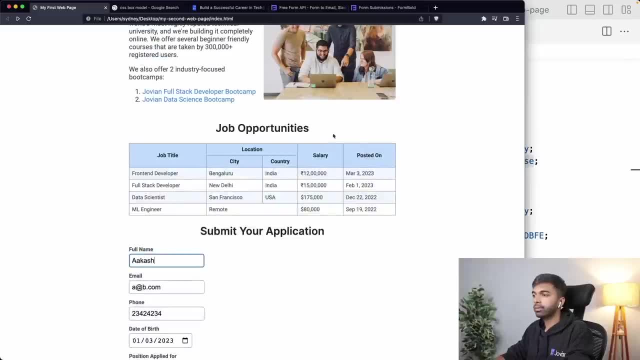 just something to Keep in mind. you can always look it up. Then we also wanted to make the table full weight, so that it occupies the entire width of the parent element, which itself is limited to about 800 pixels at the center of the screen. 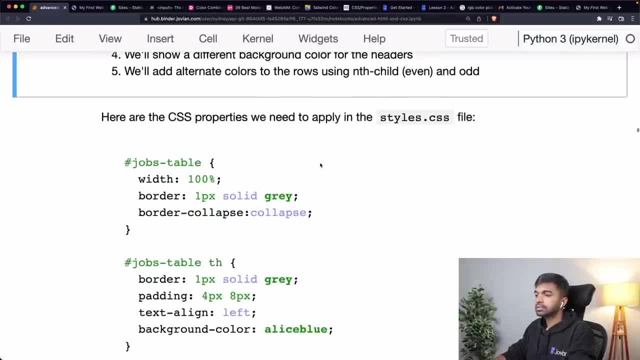 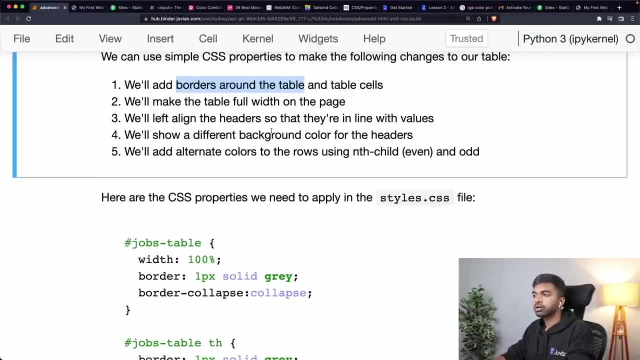 If the browser is large enough. So then we also left align the headers initially and then we centered align them again over time. Then we also try to show different background color for the header rows and different background colors for the alternate rows of the table. 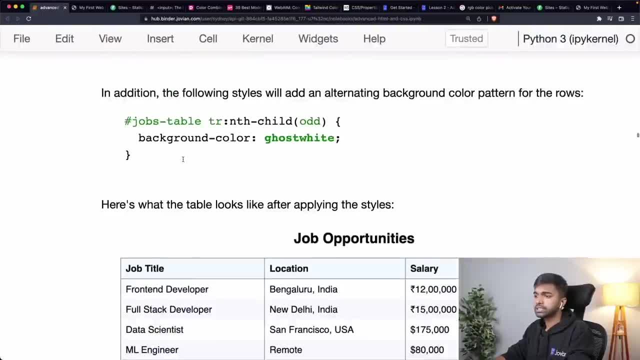 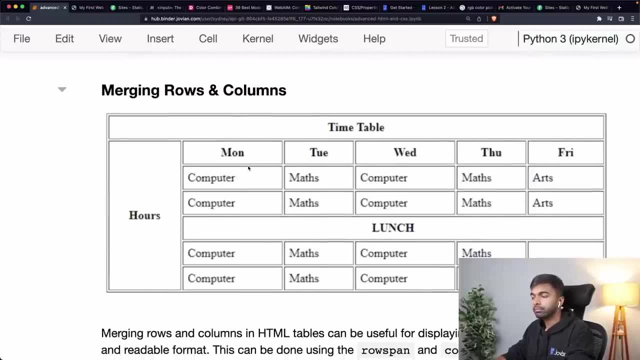 And we also wanted to make the table full width so that it occupies the entire width of the parent element, And that is all achieved using CSS, And this is what our output looked like. Then we went ahead and we looked at some advanced table row and column merging using the row. 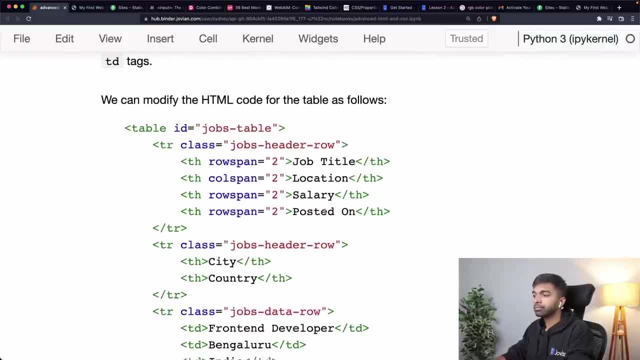 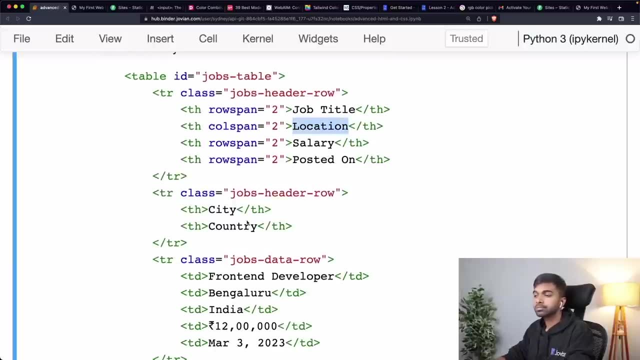 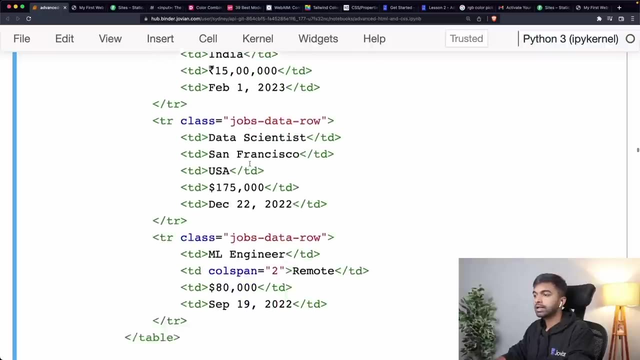 span and call span. specifically the job title, salary and posted on were configured to span two rows and location was configured to span two columns. And then we added two sub columns, city and country, under location, And then we also split the uh, the data itself, into city and country, except for remote where 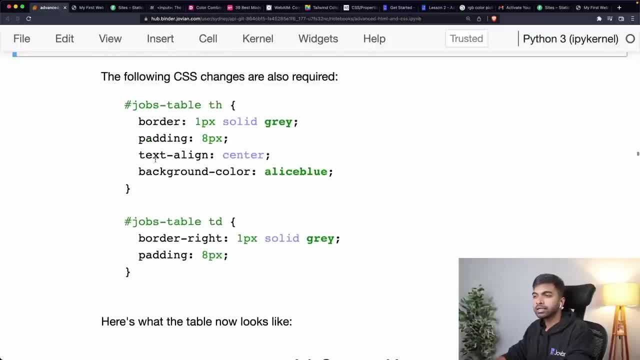 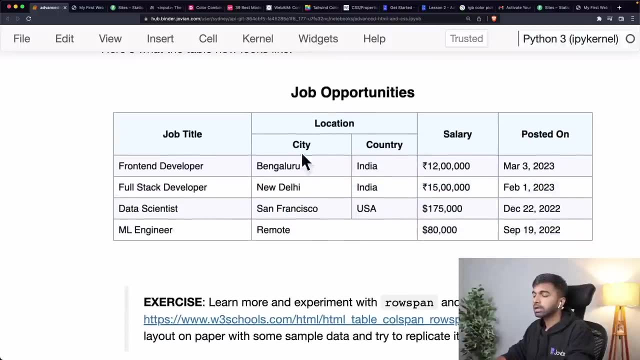 we just set it. We set it to span two columns And we also modified the CSS size a little bit to better represent the data in this new structure. So this is what our table looked like after styling. Then we learned a little bit about textiles and CSS. 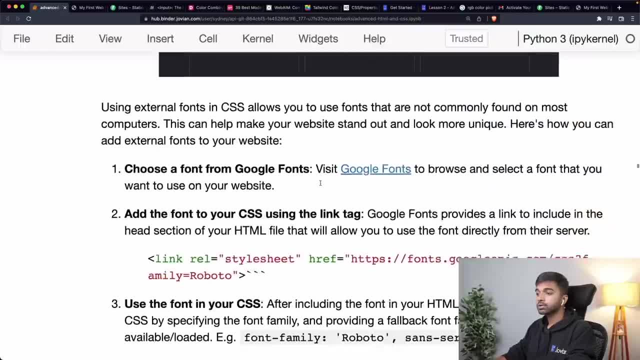 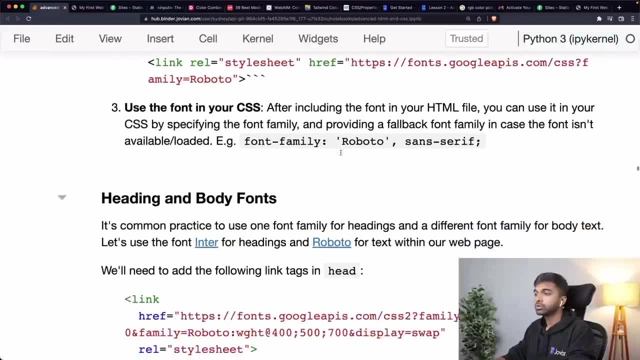 We learned about how to use external fonts from Google fonts. So you choose a font on Google fonts, You add those fonts. So you select a bunch of fonts and you add them to your CSS And then you use that font in your CSS using font family. 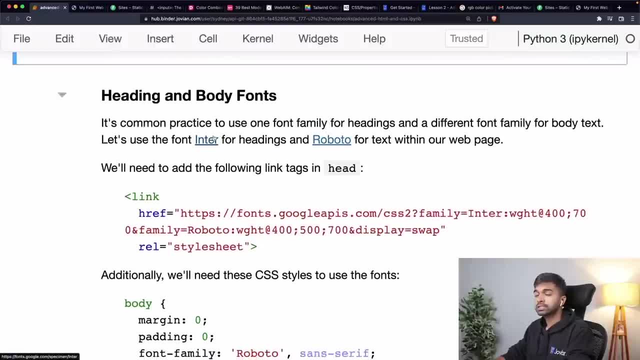 And we use font family. Okay, So we use the heading and body fonts. specifically, We use the inter font for our headings- That is what we use at Jovian- and the Roboto font for body. You can use any other pair. 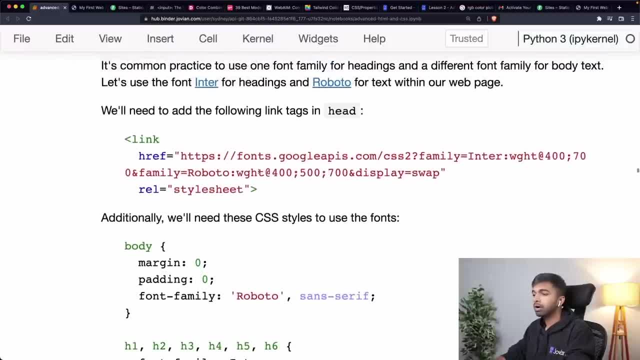 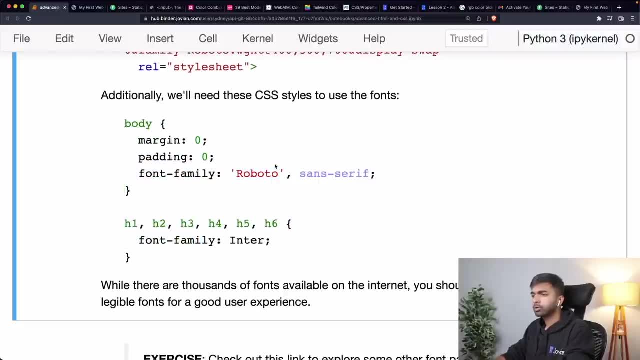 There are a bunch of pairs you can find online and to add them to our webpage We simply need the need these link tags And additionally, we also need these CSS styles, um to use these fonts. So within the body, we've added some fonts and then, for um, I added the Roboto font. 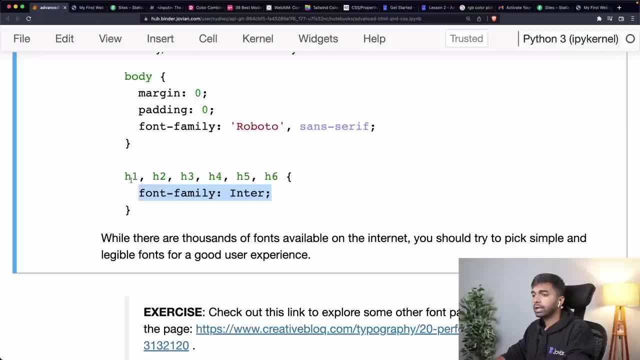 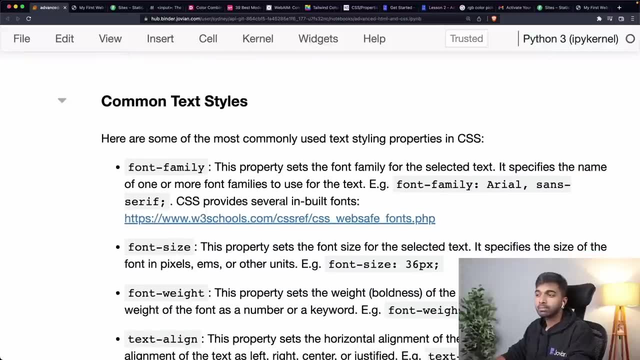 family and within the Okay, Okay, H1 to H6.. So within the headers, we have used the inter font family. Okay. Then we saw some common text styles, some common text CSS properties, Of course, this font family. then there is font size and there are various ways to express. 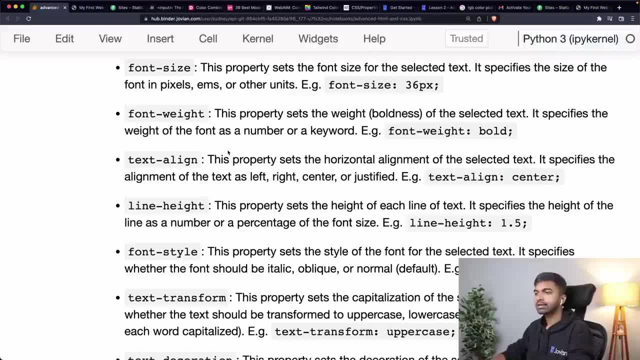 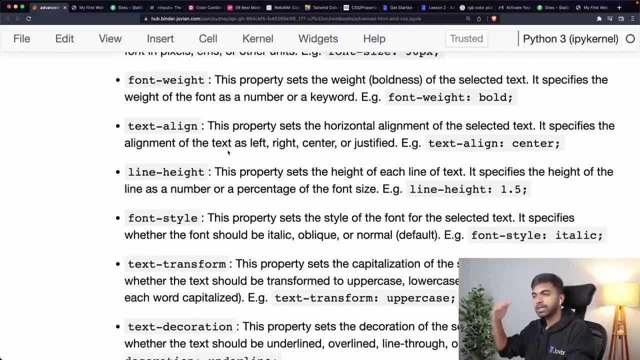 sizes and CSS. There is font weight, which is how thick each character is, So you can use 400,, which is normal, or 500,, 600,, 700, 800.. There is line height, which is how much space there should be between lines. about 1.2 is. 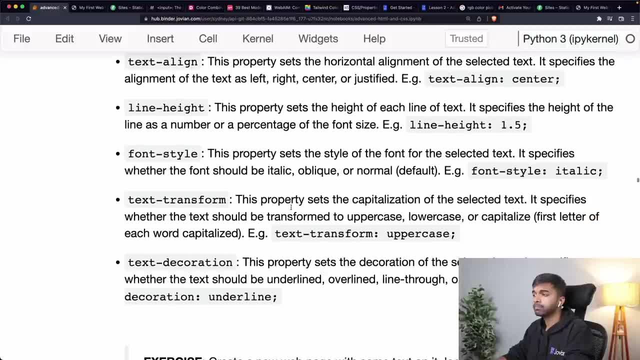 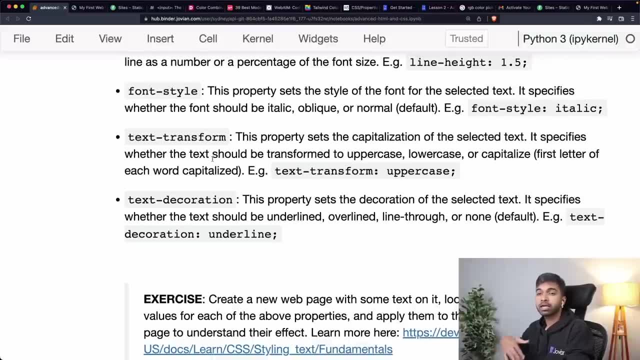 common, but you can go 1.5.. You can go smaller as well. Okay, There is font style, which you can use to italicize the text, and you can check out other properties as well. There is text transform. You can make everything upper case. 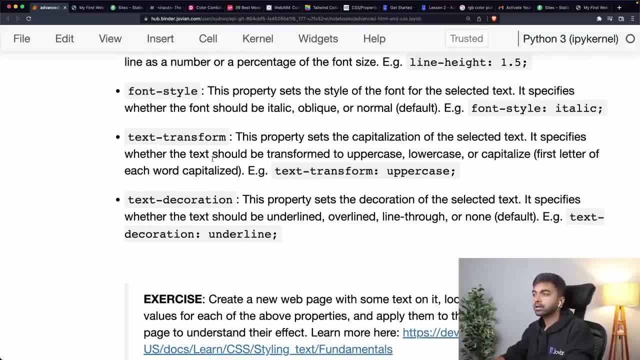 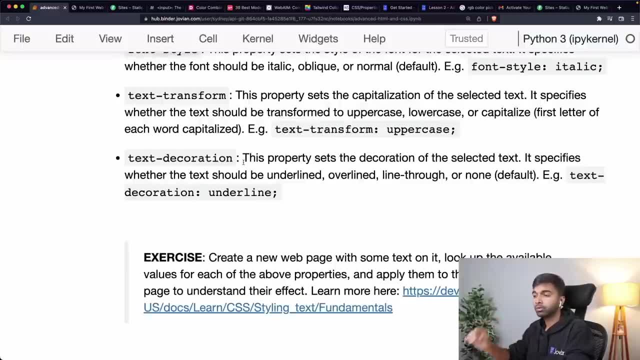 You can use sentence case, which is to capitalize the first letter of every word, or you can use a lower case, And there is text decoration, which can be used to underline, overline or strike through text. Okay, Again, you have to experiment with these and only then you become familiar and you don't. 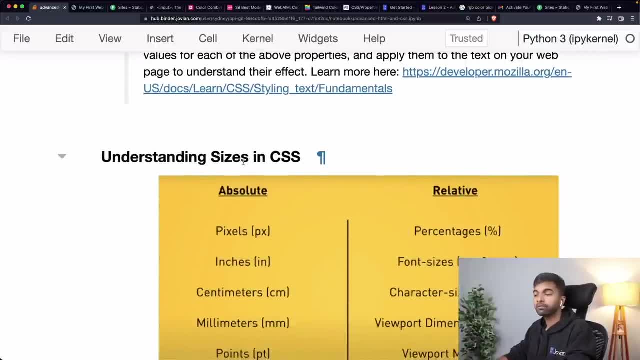 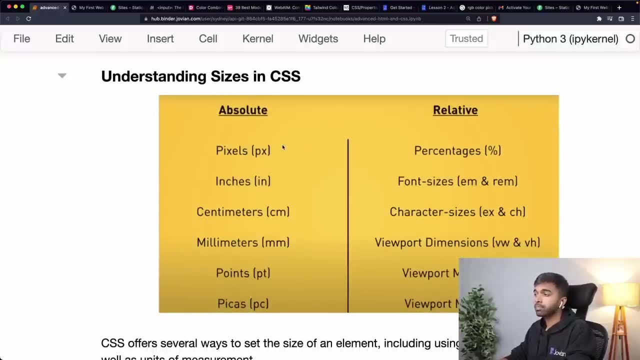 have to remember them. You can always look them up. I don't remember them after 15 years of web development. Then we looked at how to express sizes in CSS. So we have these absolute sizes, or pixels, and we have a bunch of other absolute sizes. 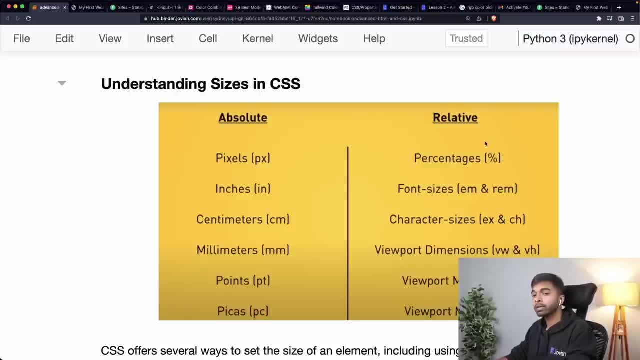 which are not commonly used in relative sizes. Percentages are more common when we are specifying weights or heights for divs, but for fonts we often use M and REM. M expresses the current elements. font size as a fraction or a proportion of the parent elements. font size and REM. 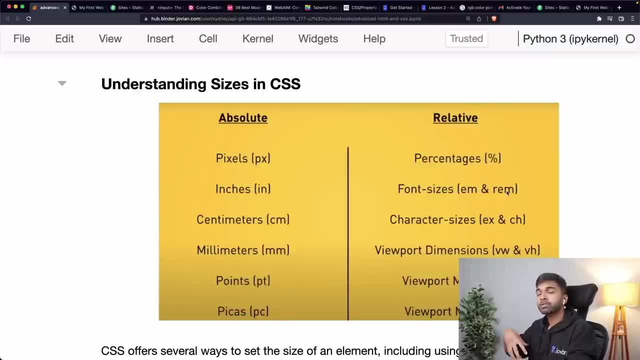 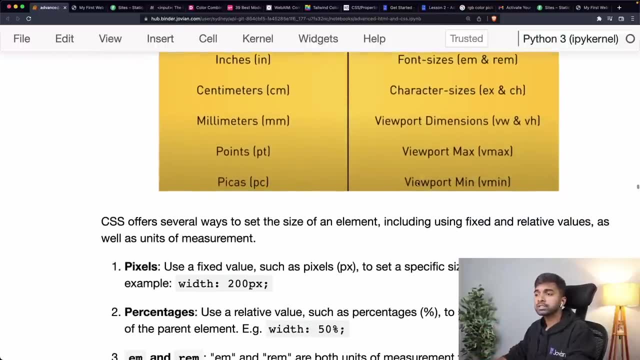 Okay, It also expresses the current elements font size as a proportion of the default font size for the entire page, which is set on the HTML tag, I believe. Okay, There's also these viewport dimensions. that is left as an exercise for you in terms of. 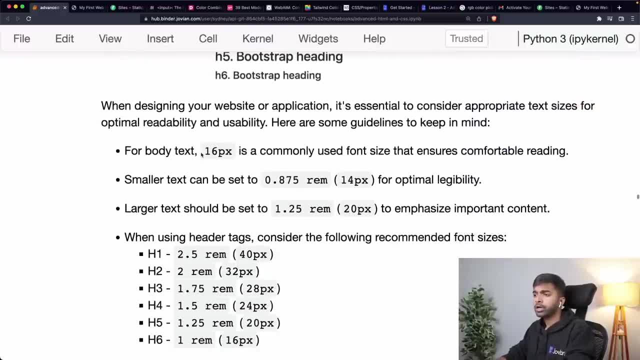 sizing We had some guidelines: that for body text 16 pixels is a common size and smaller text can be 0.875 REM or 14 pixels and larger text can be a 1.25 REM or 20 pixels. And then for headers you can use different sizes from 2.5 REM to 1 REM. 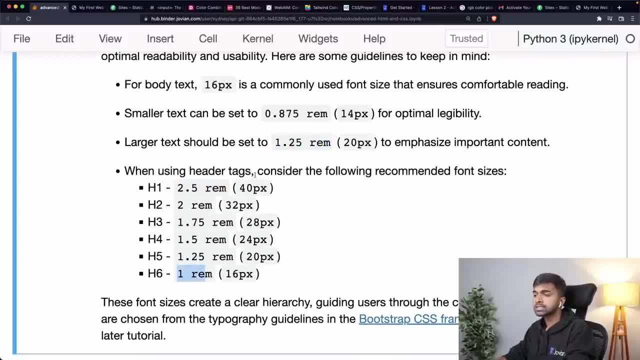 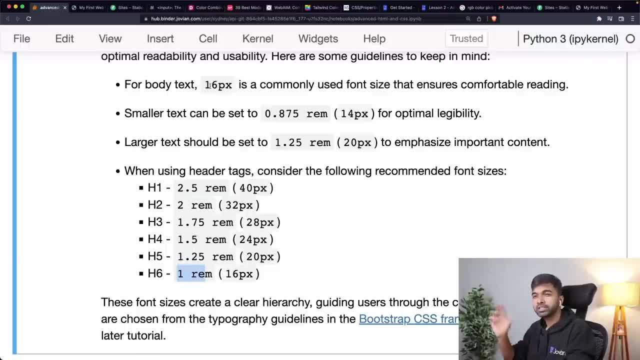 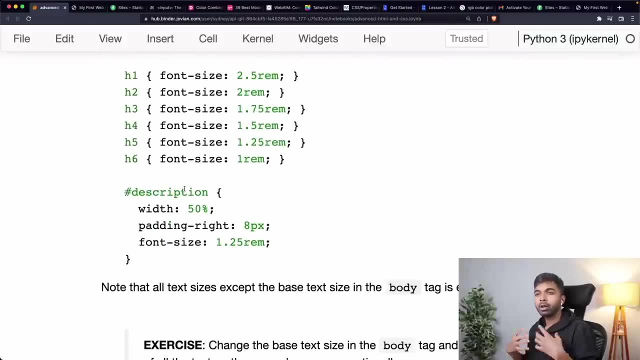 And we prefer using REMs for sizing, because you can simply go and change the HTML tag text or the root text of the body of the page and everything will get updated automatically. And then you can, of course, specify these styles in CSS. So, again, type out all the code yourself. 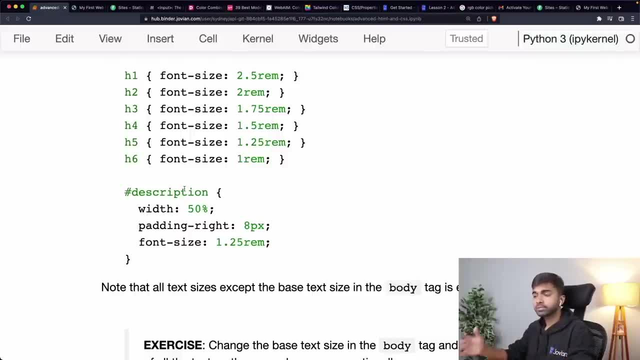 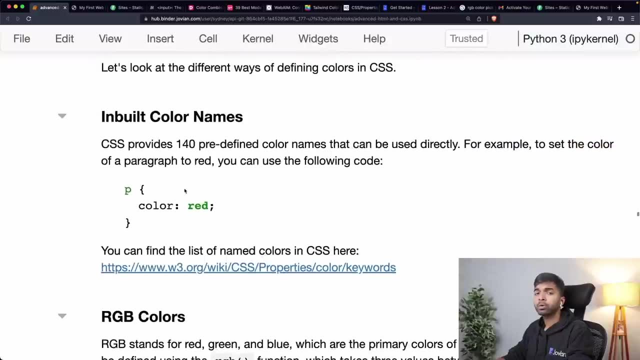 That is how you understand this. You should spend four, five, six hours this week just typing out all this code on your own. Then we looked at some guidelines around colors. The first thing we looked at was how to use colors in CSS. 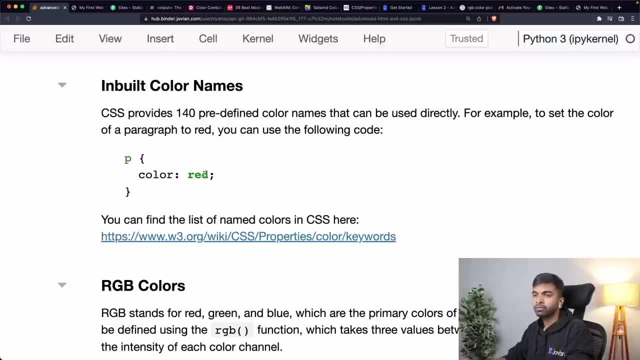 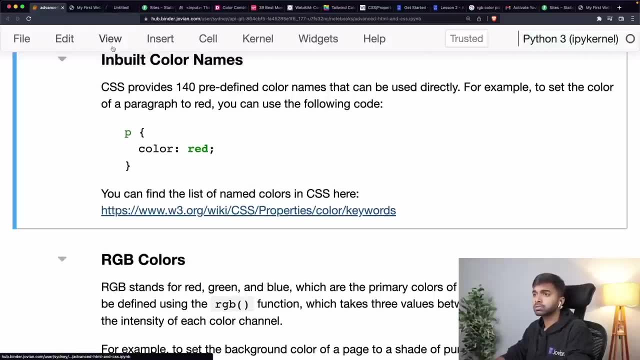 Of course we have a bunch of inbuilt color names, but often you will find that they do not look very good when you actually use some of these inbuilt color names. but you have a bunch of these you can use from and if you want to use an inbuilt color, start with. 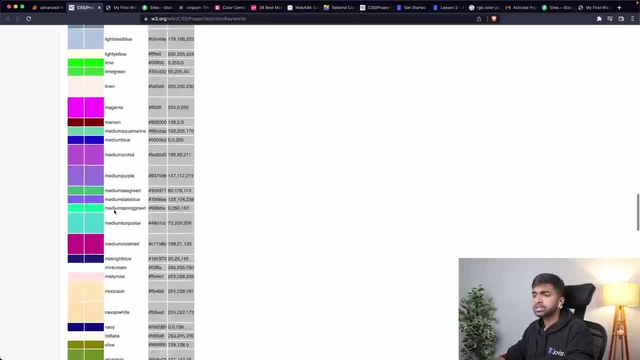 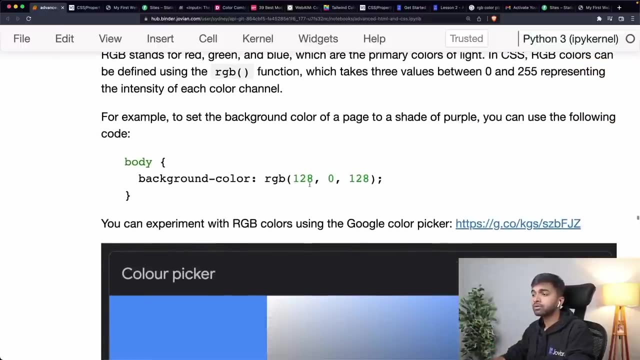 a color that is very muted, very light, So maybe just a light, the last set of colors here- And of course, you can use RGB- red, green, blue- and you can specify a value of zero to 255. For red, green and blue respectively, and that is going to create a color for you. 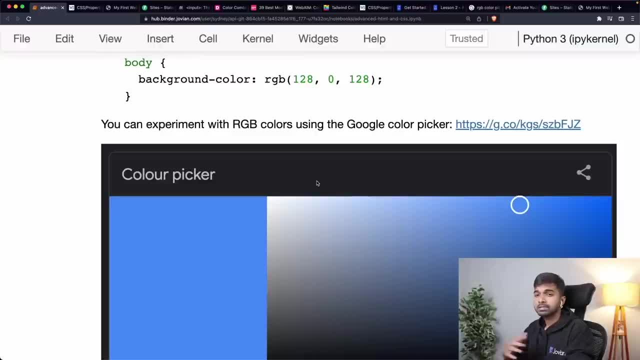 Zero is dark, 255 is light. So you can go from black to white. If you vary all of them equally with grays in between, or if you pick different values for red, green and blue, you can create millions of color combinations. 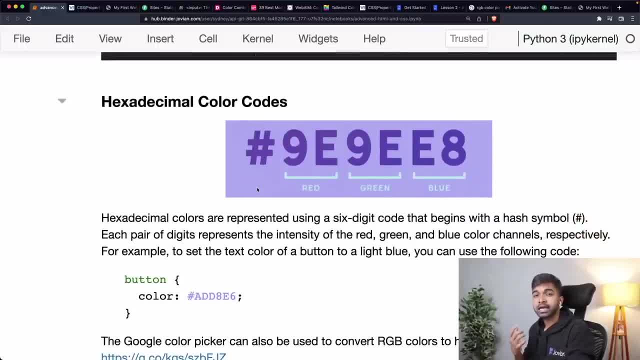 Now, another way to represent red, green, blue colors is using hexadecimal codes, and this is the hex, or the base 16, representation of red, green and blue combined together into a single string, And this is what you often find on the internet, because these are easy to copy and paste around. 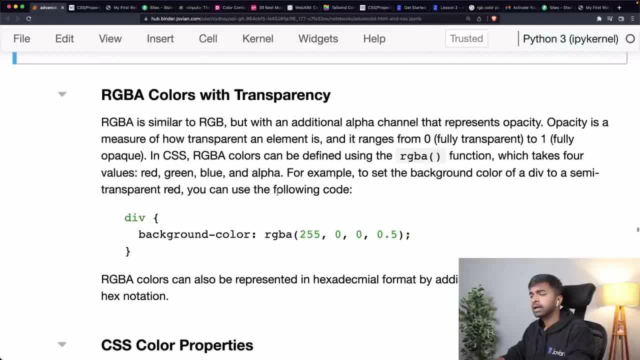 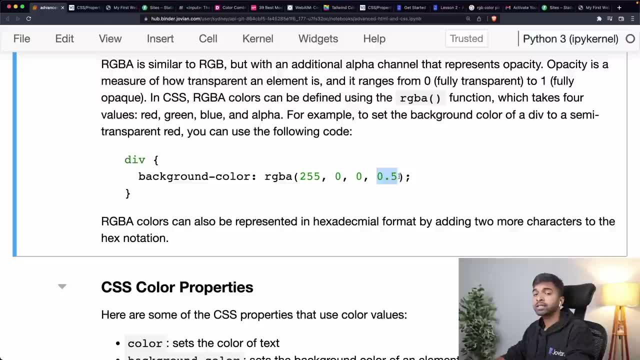 instead of RGB. And then we have RGB colors with transparency, So you can use RGBA, where you can specify red, green, blue values and you can specify the opacity value. One is completely opaque and zero is completely transparent and 0.5 is somewhere in between. 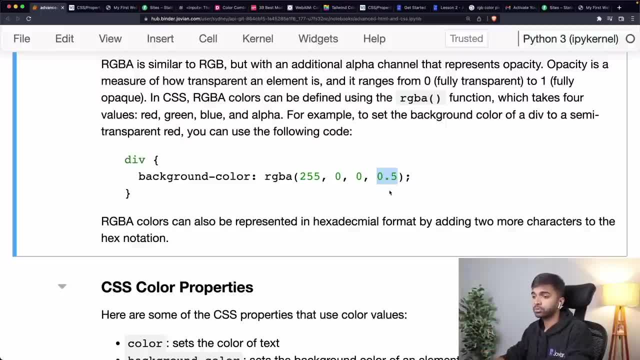 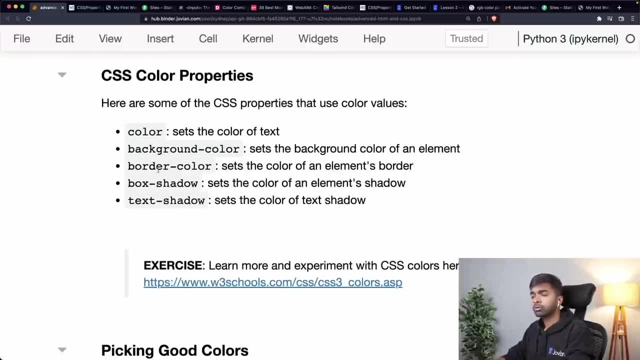 So that the background color is going to show through or the background image is going to show through. Then we have CSS color properties So you can use color, background color, border color box shadow, text shadow, all these properties that have color. 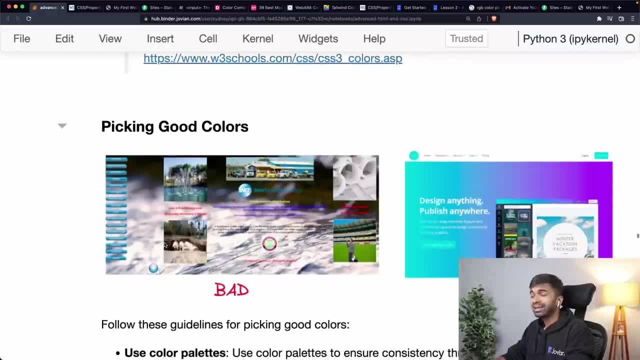 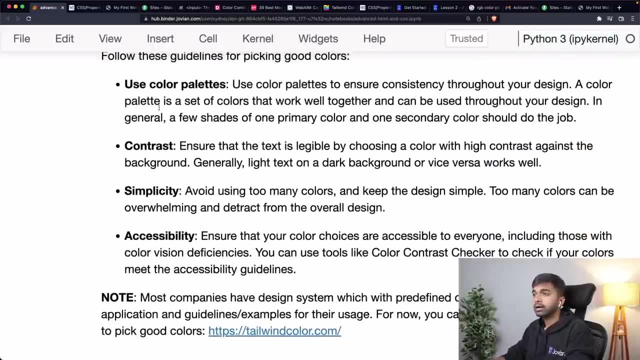 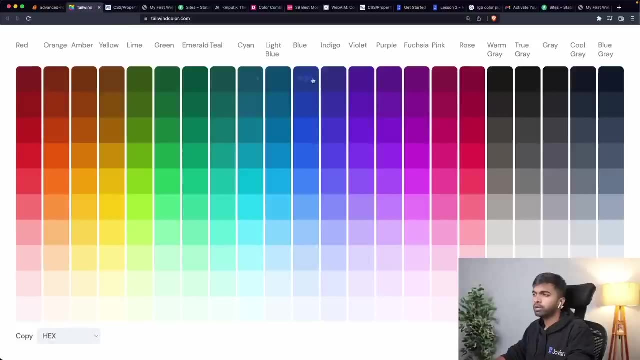 And there are some other properties as well that can use color. Okay, In terms of picking good colors, ideally you should be using color palettes. You shouldn't be picking random colors from the internet here and there. A good color palette tool is Tailwind colorscom, where you can just use maybe one of these. 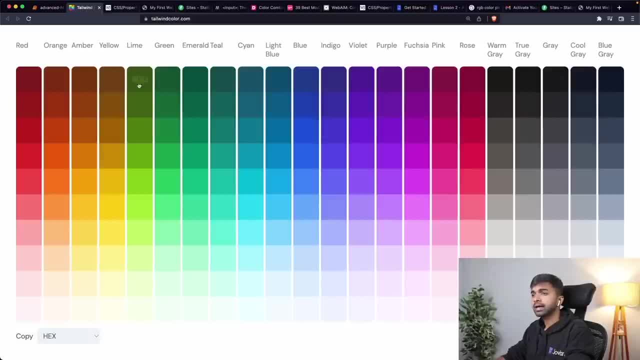 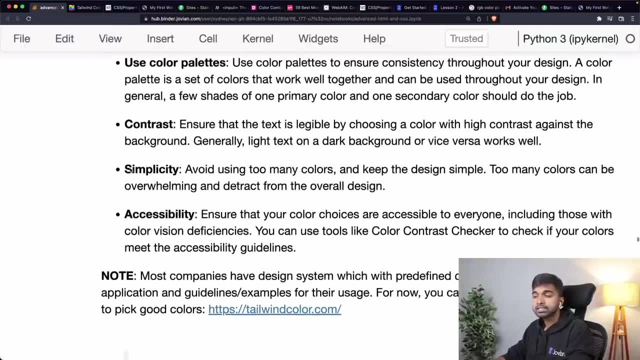 as the primary color and then use a bunch of grays for text And maybe a secondary color. If you need to use a second color, Okay, And just use shades of the same color. Also, have enough contrast. Keep it simple. 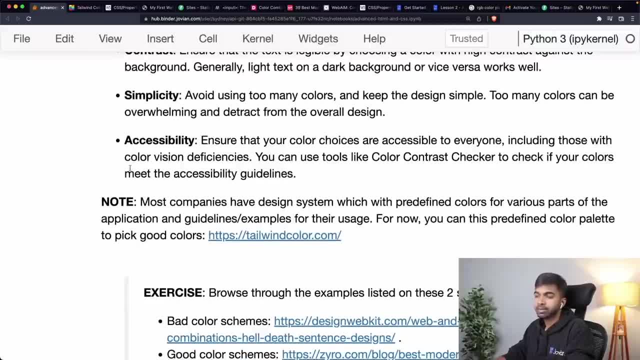 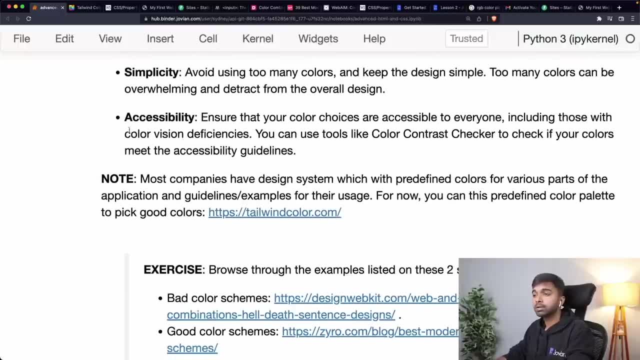 Don't use too many colors. and don't use colors just because you can. sometimes black over white is as good as it needs to get. Also, make sure that the colors are accessible to people with color vision deficiencies. Okay, There are some examples of good and bad color schemes that you can check out in general. 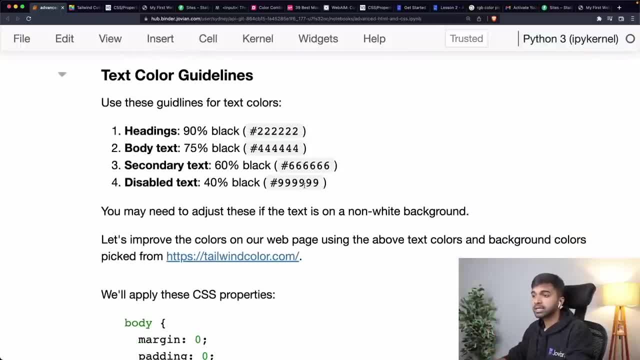 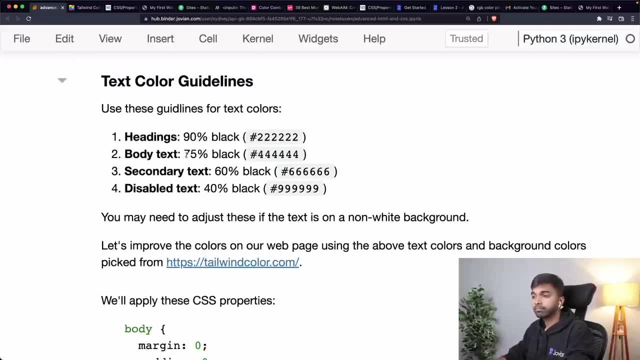 It's a good idea to maybe explore the color schemes of specific websites and for texts, specifically For headings, you can use 90% black with a tinge of blue or green as per the website that you're on, that you're designing, or body text. 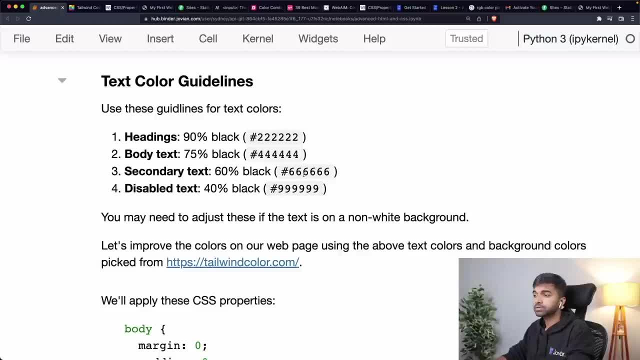 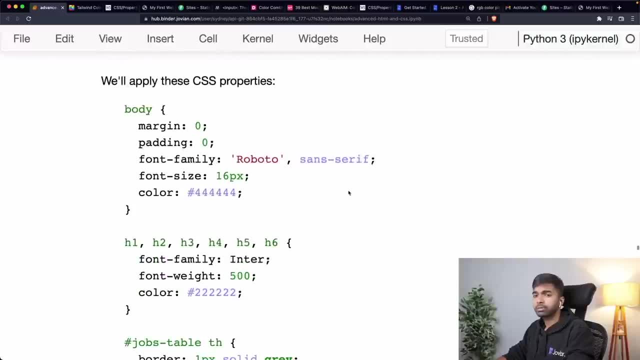 You can use 75% black or four, four, four, four. for secondary texts, You can use a 60% black and for disabled texts, you can use 40% black. So these are good rules of thumb to make your pages look good. 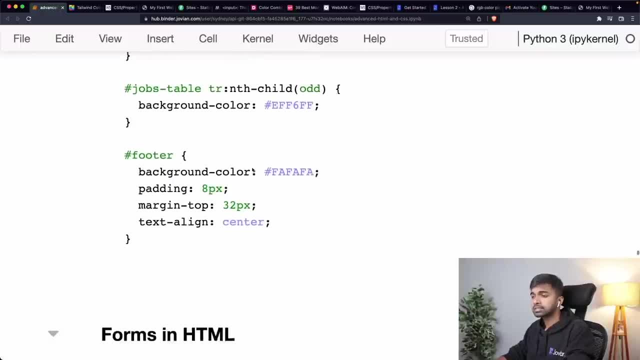 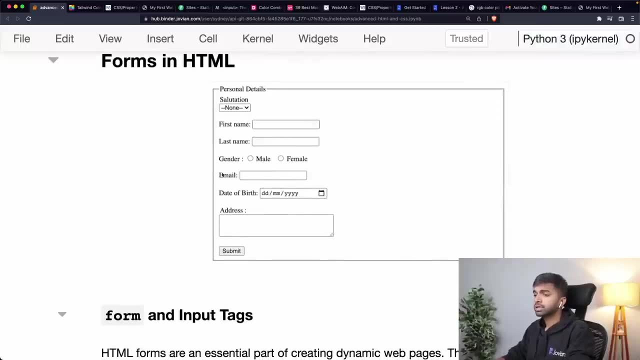 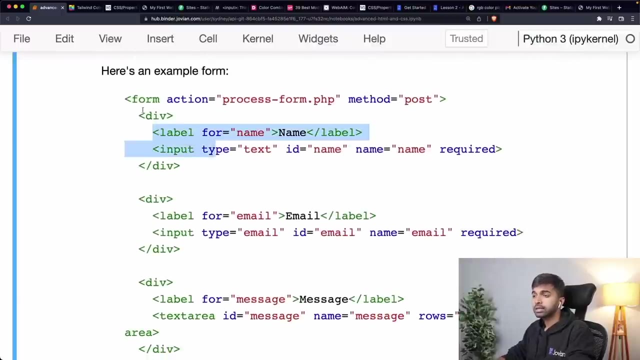 And we've just applied this to the various headers and the various headers, footers, etc. in our code. Then we looked at forms in HTML, so you can create forms using the form tag, And in the form tag you can then specify labels and inputs, and inputs can have various. 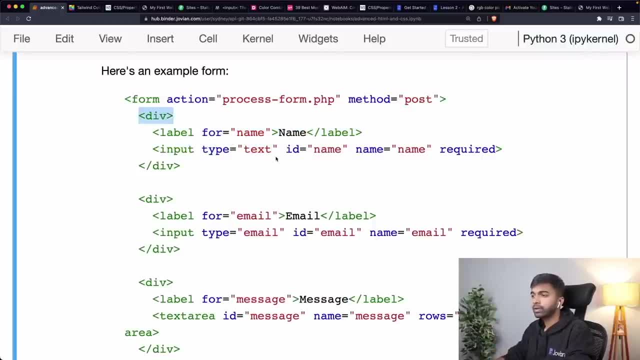 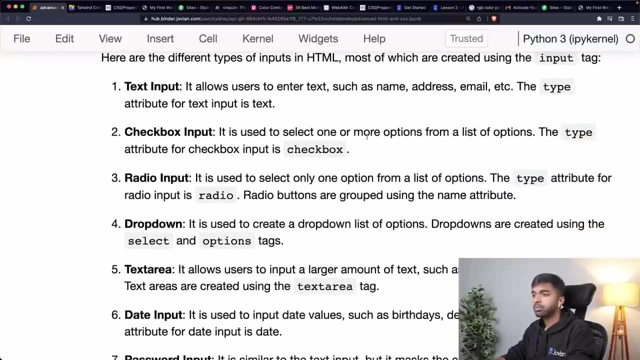 types And normally we put these within divs so that each shows up on a separate line. And of course you can also add a BR tag after each label to show the input on the next line after the label. And there are various types of form inputs: text, checkbox, radio dropdown. 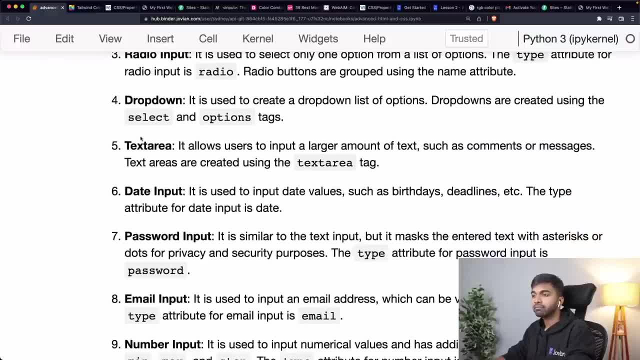 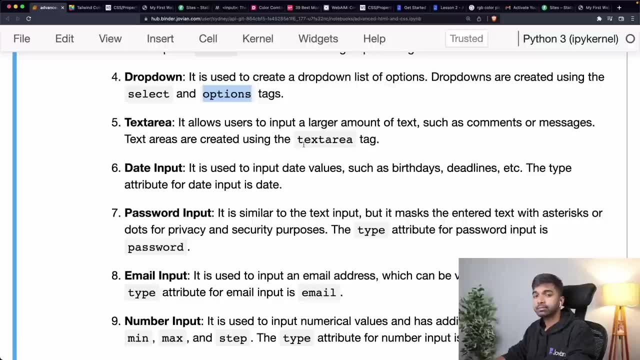 So most of them use the input tag. Some of them use a different tag. For example, there's a select tag- Okay, That's used for creating dropdowns- along with the option tag, And then there is the text area tag, which is not a self-closing tag. 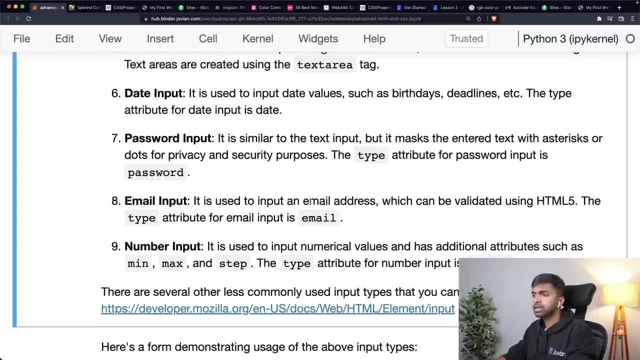 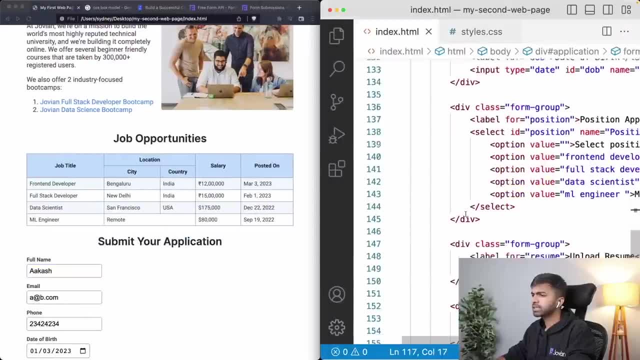 That's one thing to remember. And we have data input, password input, email input. These are again all inputs, and we have number inputs as well. So then we created this actual application form here, which was which had a bunch of. 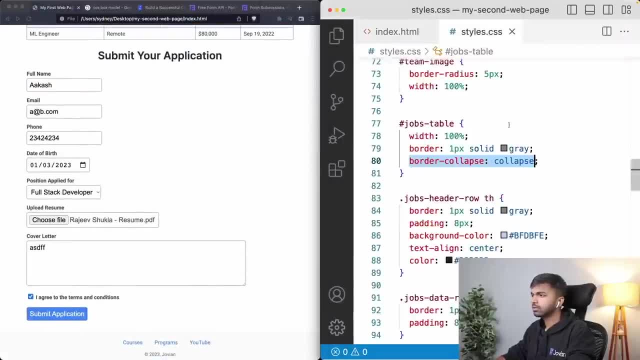 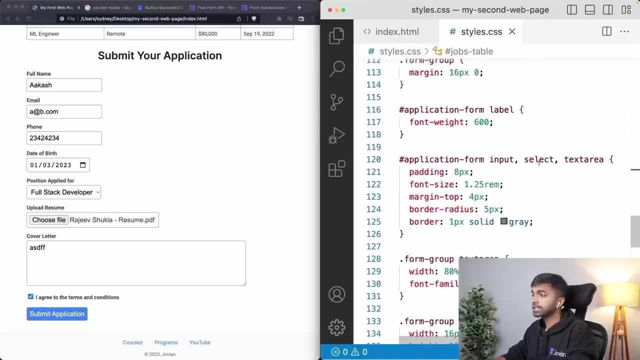 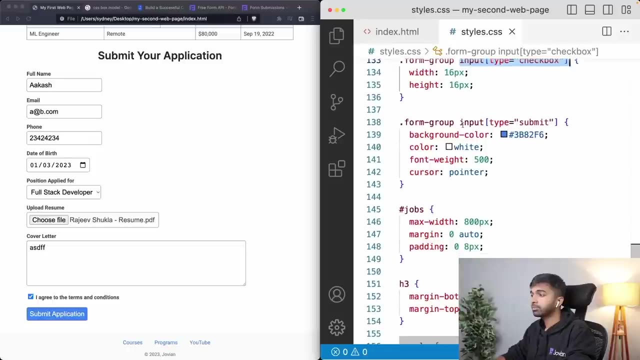 fields and we also styled it using CSS. So we looked at some various interesting ways to select things. So, for example, we selected the label changes font weight. We selected the input select text. here altogether We selected input of type- checkbox using this special kind of selector, and input of type. 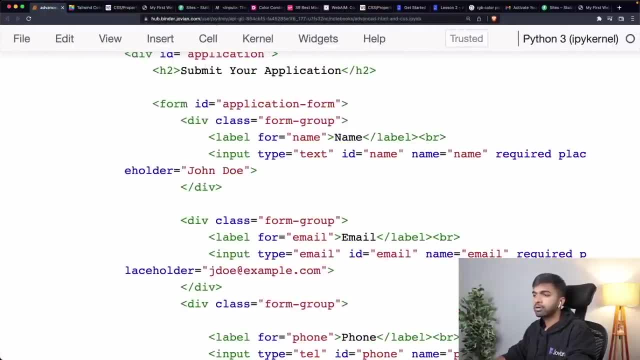 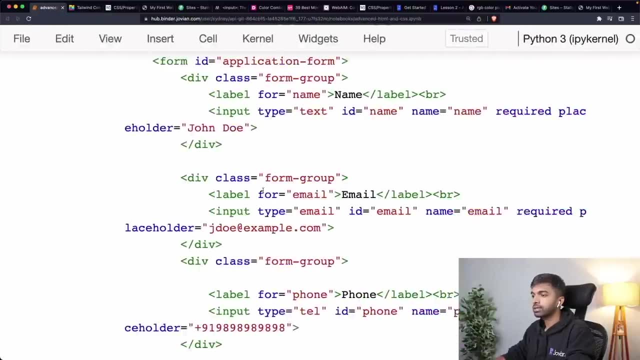 submit, which is a submit button using the special kind of selector. So you have all these interesting ways to select and style forms, And over time we'll start using frameworks, So you won't have to do much of this styling on your own anyway. 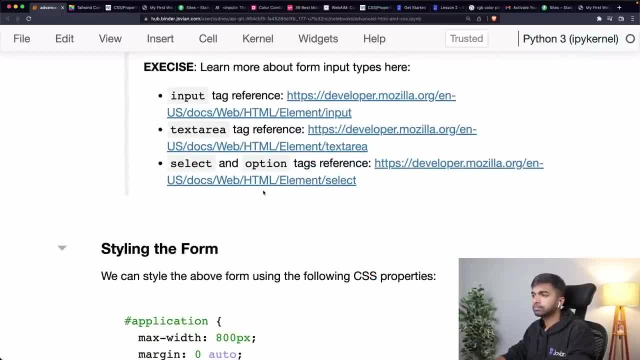 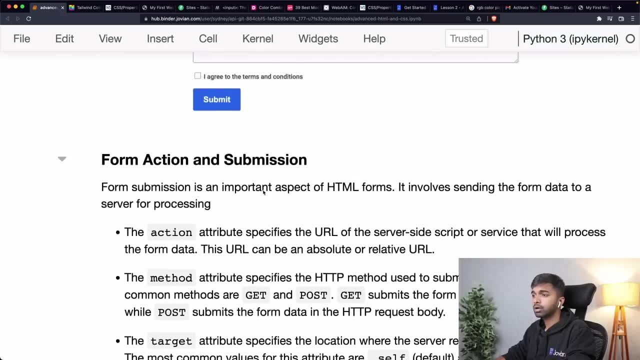 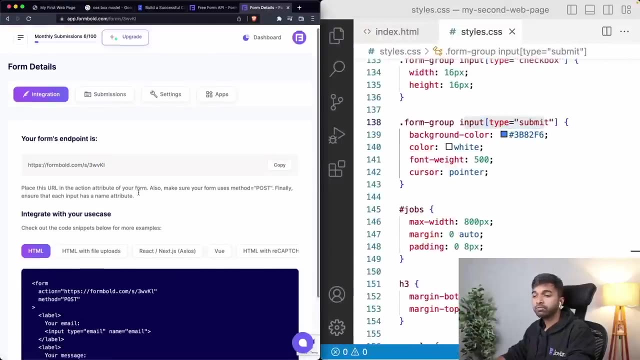 And finally, once we did all that, we also then deployed this website to. we also then used an online platform called Formcom- FormBold. So we signed up on FormBoldcom and we created a new form inside FormBoldcom, copied the. 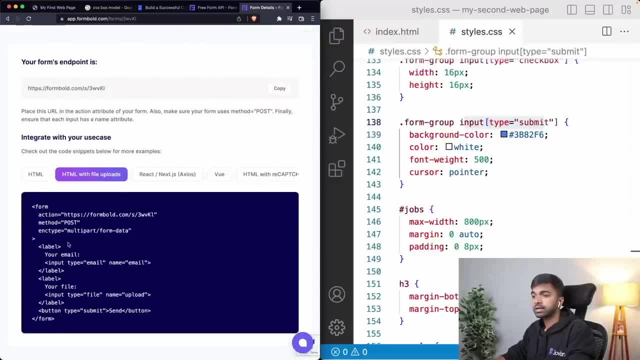 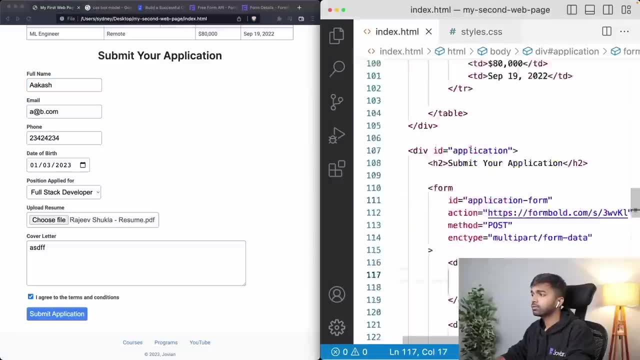 action that we need to set up into our form, And we have some example text here. so we need to put the action method and, apparently, this ink type into our form, And what that does is when the user hits submit, this data is going to be sent to this site. 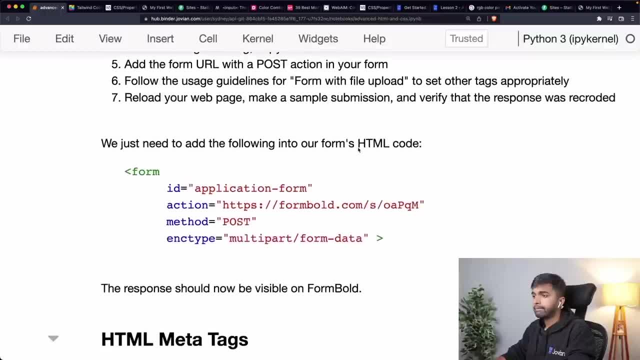 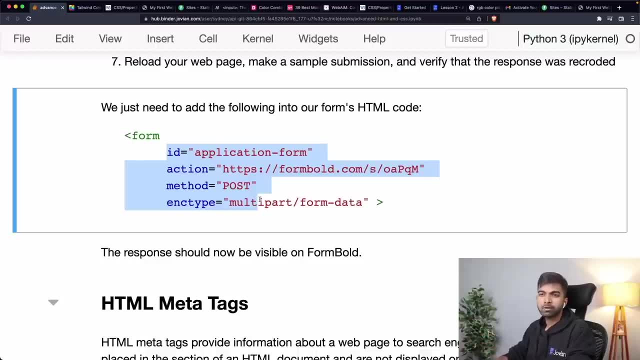 called FormBold. Okay, And that's it. So we just need to add these few lines and we can send our form data wherever we want. It can be a completely separate site, but over time we'll, of course, build our own server. 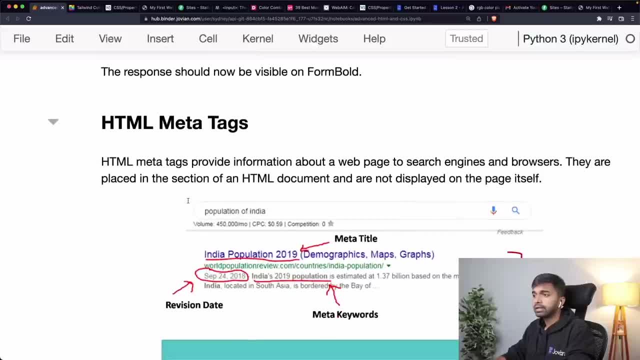 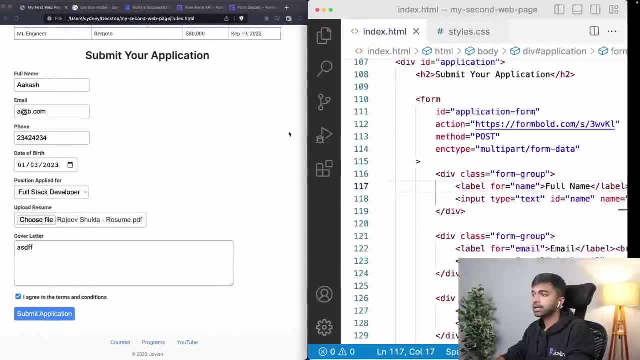 which is going to accept this form data, And that's what we looked at. You can check out the section on HTML meta tags if you need. And finally, deployment was really straightforward. All we did was create a zip file, and that's a file contained our indexhtml stylescss. 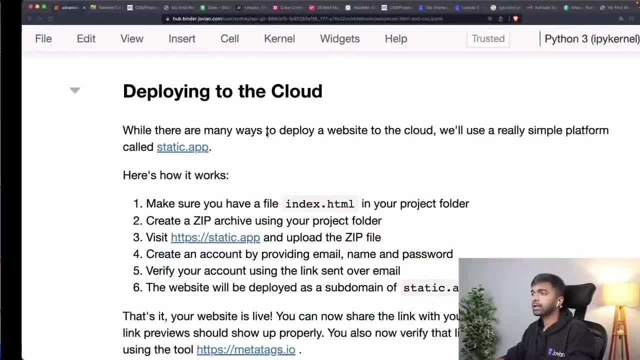 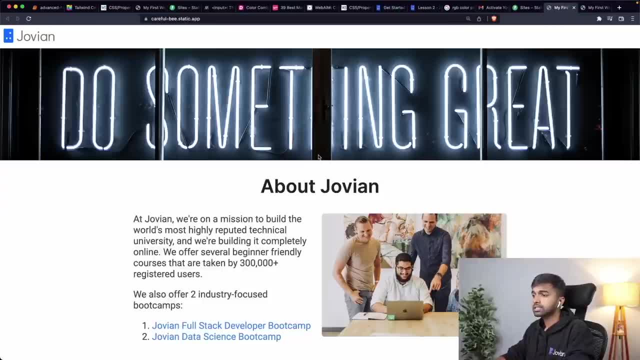 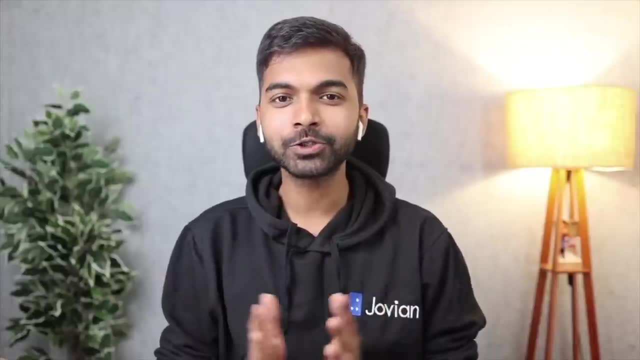 team and bannerjpg files, And we took that zip file and uploaded it on staticapp. and when we uploaded it on staticapp, it created this free site for us and in this free site we simply deployed it and we tested it out. Hello and welcome to this live workshop on turning a Figma mockup into a web page. 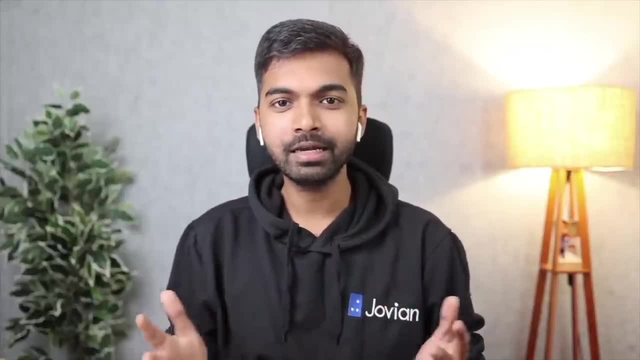 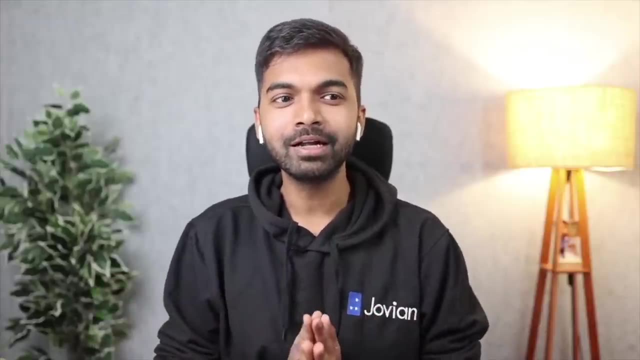 And this is completely unscripted- I'm going to pick up a design and I'm going to implement from scratch something that I've not practiced before. So you will see me making a lot of mistakes. You will see me. You will see things go wrong. 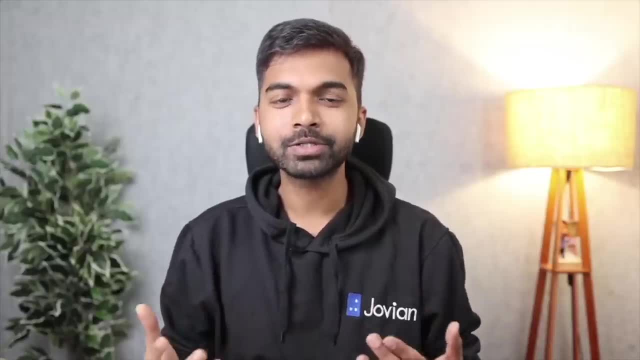 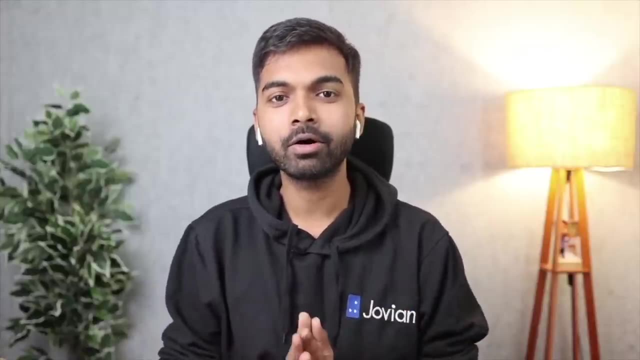 But I hope to show to you, Okay, What happens when you are going through the process of turning a design into a proper web page, What are the challenges you encounter And how can you answer or overcome some of those challenges. So with that, let's get started today. 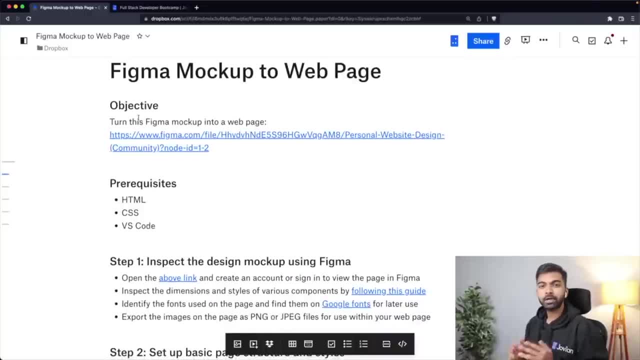 We are going to pick up a mockup from Figma. By the way, Figma is a design tool, So at most companies you will find designers. specifically, UI or user interface designers use a tool like Figma to create mockups of web pages. 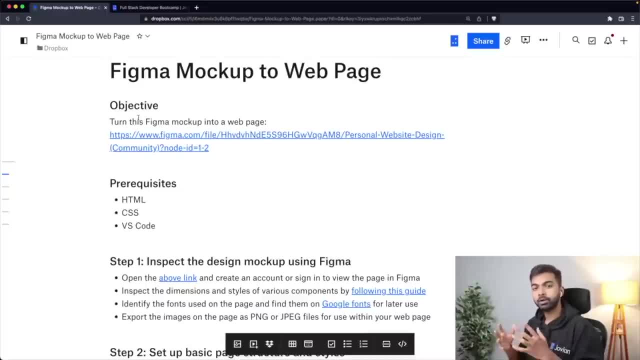 And then, as a web developer, You will have to turn those mockups into proper HTML, CSS, or sometimes you might use a framework like react, et cetera, And if not Figma. sometimes people use a tool called sketch, Sometimes they use some other tools, but every design tool more or less look similar. 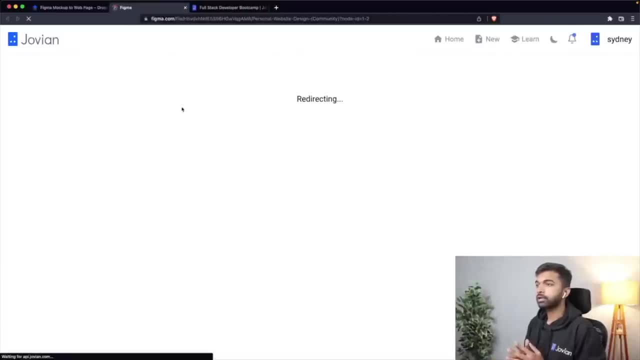 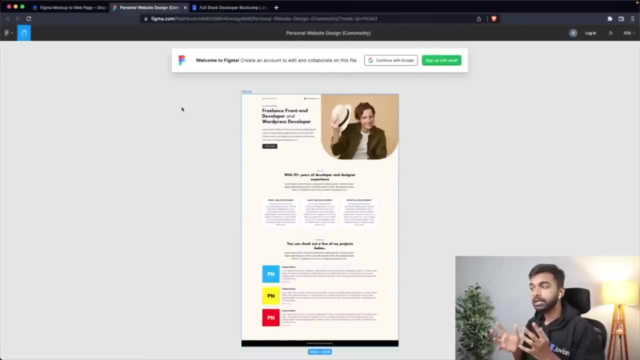 And let us open up this mockup. So typically, as a developer, you will receive a read only copy of the mockup and you are going to be able to then inspect specific areas within that mockup. So looks like Okay. So this is the web page that we've picked out. by the way, I've picked this out from 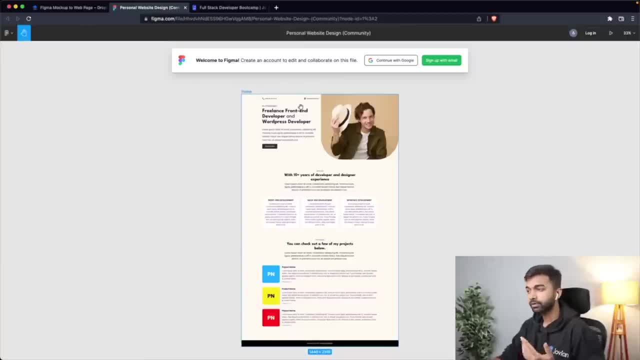 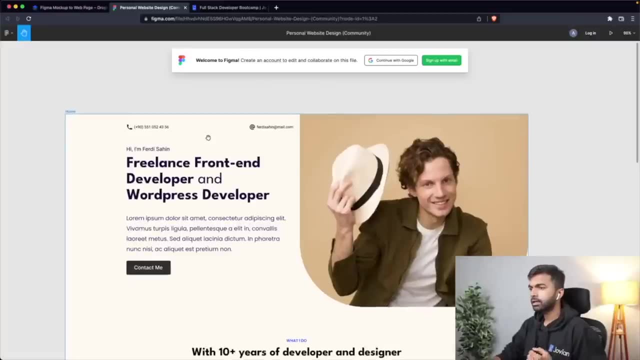 the Figma community, which is where a lot of free- to such a free- web pages can also be found, in case you want to practice, And this is what we'll try and create today. So we have this web page where this is created by Ferdy Sahin. 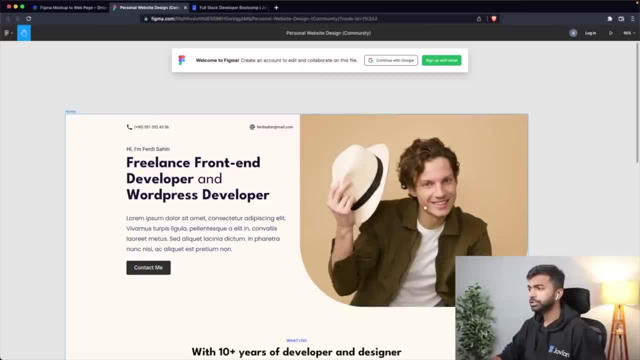 And it looks like we have their phone number, email, and we have a picture- Not sure if it's a stock picture- of it's a picture of the person who created the design. Then there is this: this is often called the hero section. 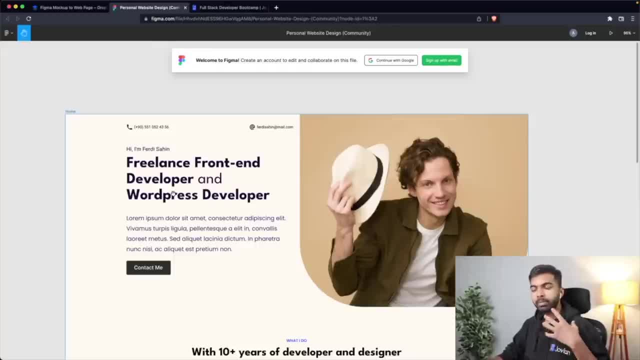 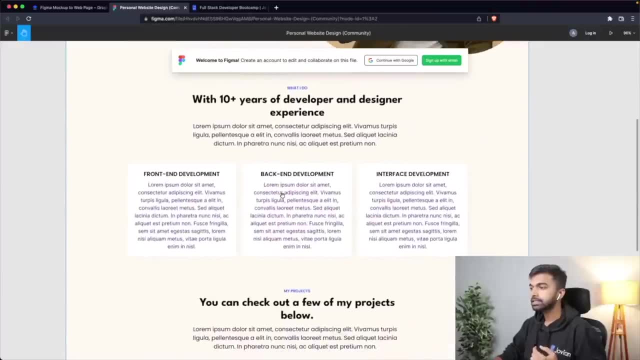 This is often called the section Where you have some big text and maybe a call to action or a button. in this case, that button seems to be contact me. Then there is a section called what I do, talking about his developer and designer experience. 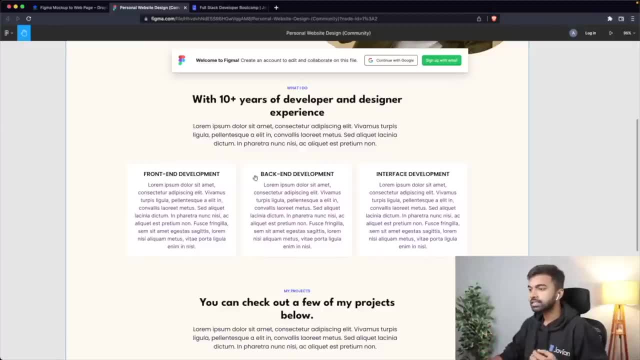 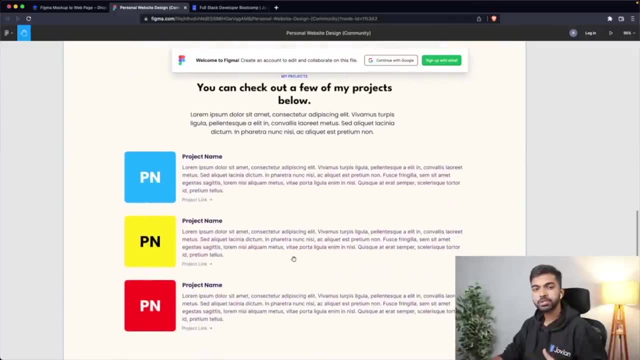 So this looks to be a personal website And there is some information about front-end development, backend development, interface development that he's talking about here. Then there is information about some of his projects and, of course, most designers will just put in some random text or lorem ipsum. 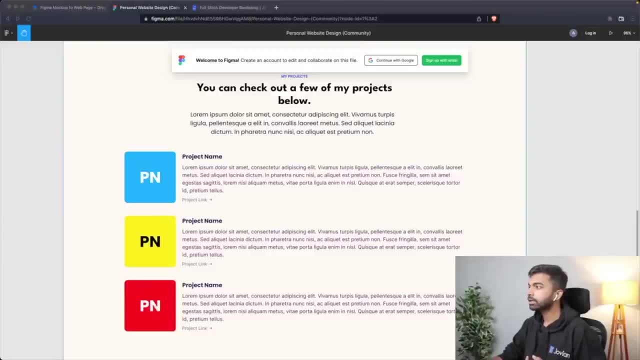 Some text, as this is called, most designers will put in a lorem ipsum or a placeholder text, But of course, in the real world, when this, when this website goes live, some actual text can come in here. Okay, So this will be information about the projects created by Ferdy. 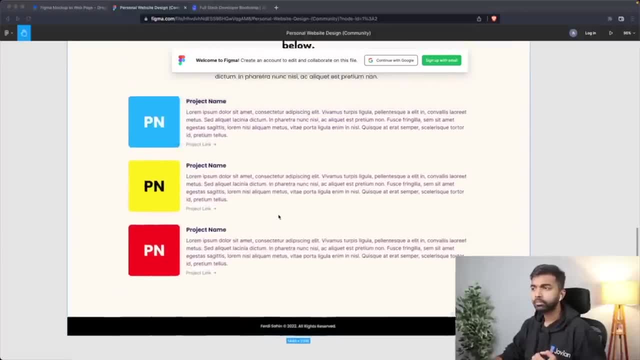 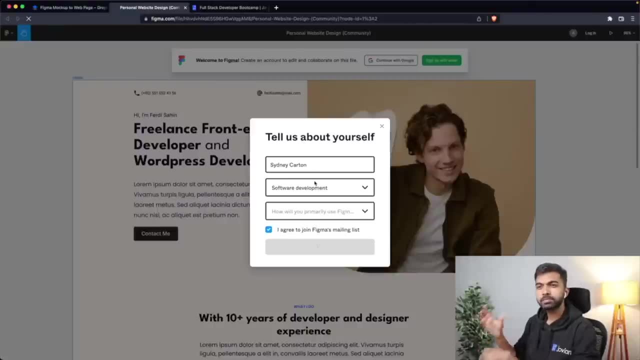 And then there is also this, a footer at the bottom. All right, There's actually a more. let me just sign up here so that we can actually see this, And I'll be able to inspect specific parts of this webpage. I'll be able to look at the fonts, colors and things like that. 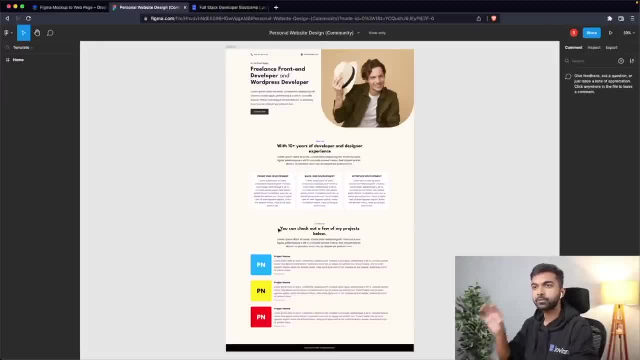 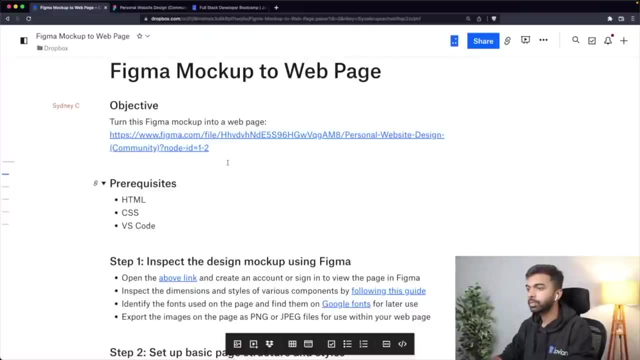 And, in fact, I'm going to pick a slightly harder version of this. So this is what is given as an assignment in one of the courses that we are running. This is, in fact, the first assignment on HTML and CSS, but I'm going to pick a slightly. 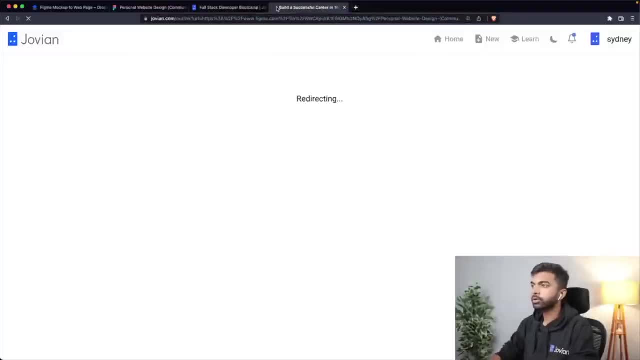 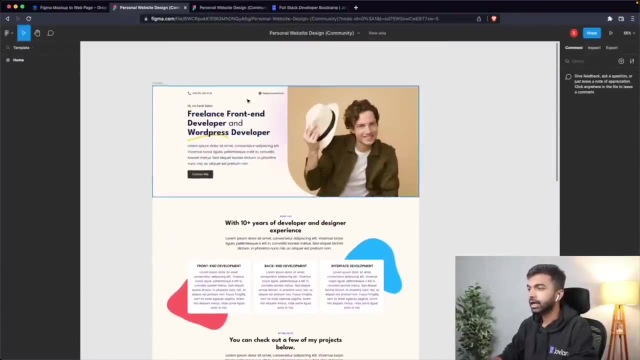 harder version of this, So let me just find that. So I'm going to use this extended design mockup, something that is actually a little bit harder. So here now we have not just the same hero section, but we also have this in this skills. 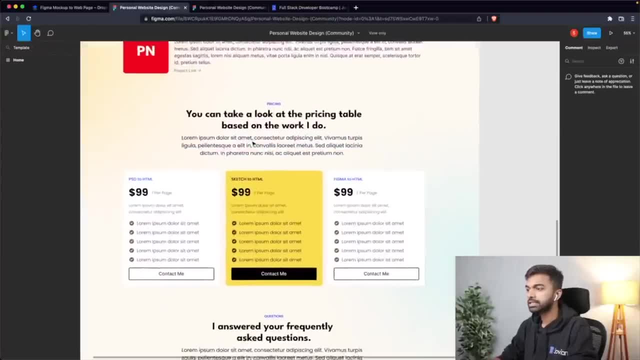 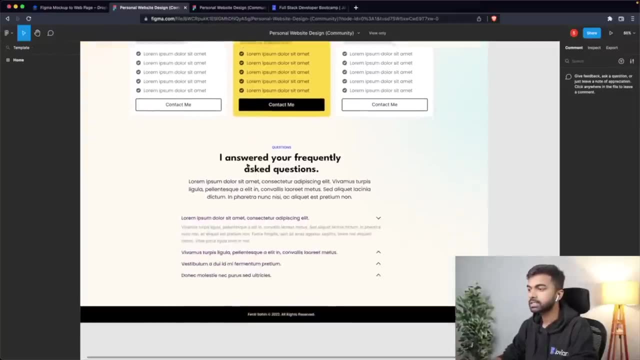 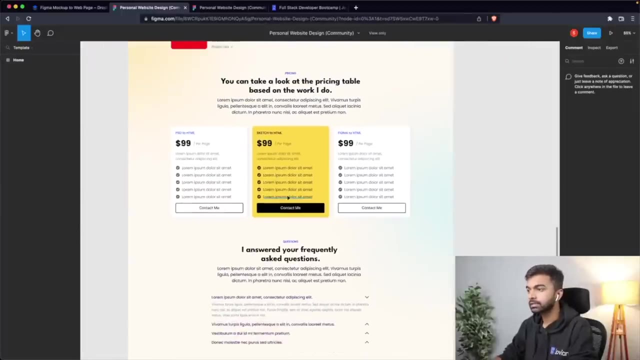 and project section, as before, but we also have the section called pricing, Which seems to have like a pricing, a bunch of pricing elements sharing information about various services, And we also have this section about frequently asked questions. So what we'll do is we'll try and cover some of these more advanced design elements as 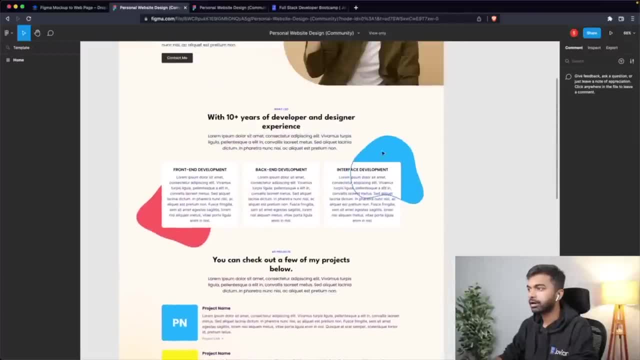 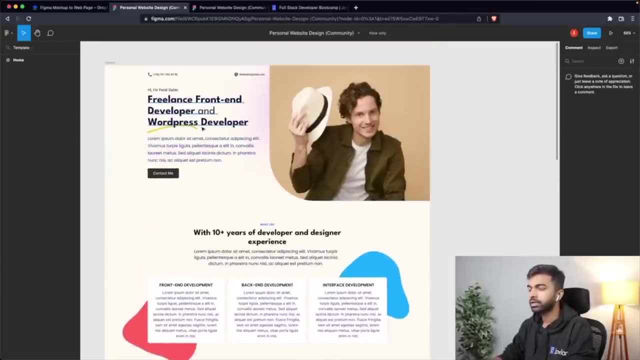 well, And maybe we'll also try and add some of these background elements. So there seems to be this background element over here, There seems to be this background element here And there seems to be this line over here that shows up just below WordPress developer. 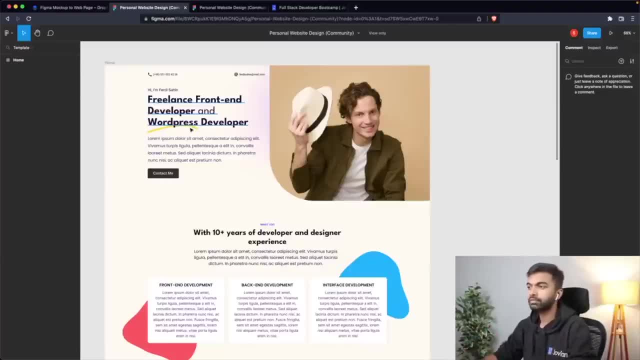 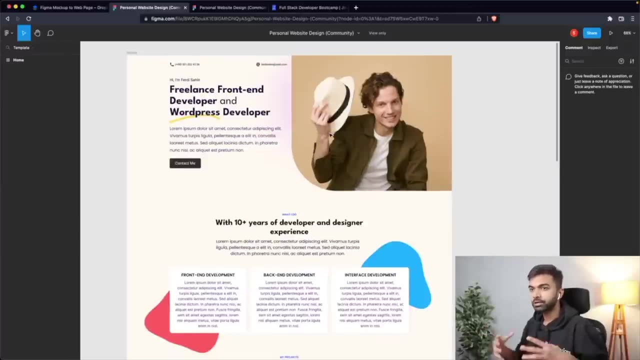 So we'll see how much of this we can cover. I have no clue if we'll be able to touch on all of this within the hour or so that we have, But whenever you're given us a design mockup, this is where you should start. 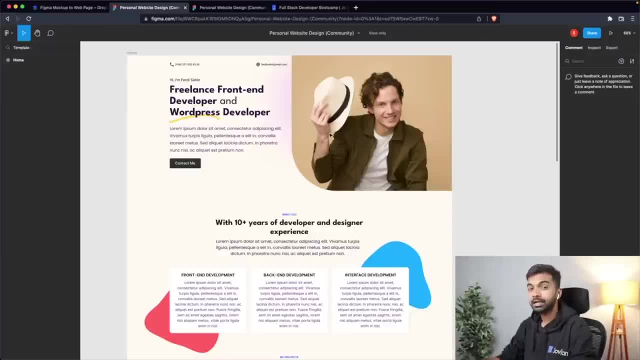 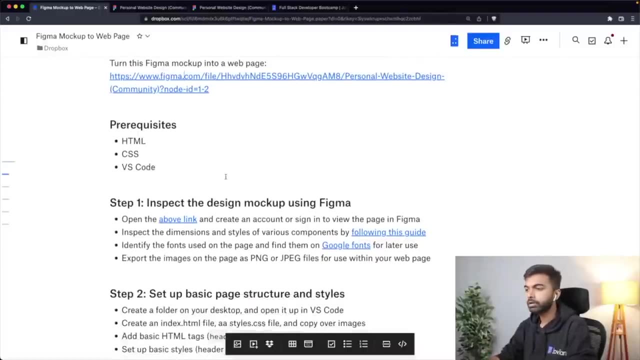 You should start by just starting the page and understanding what's on it, identifying the various sections within the page, And I've actually laid out a step-by-step process that we will try and follow today very, very roughly, But the prerequisites that I'm assuming here are HTML. 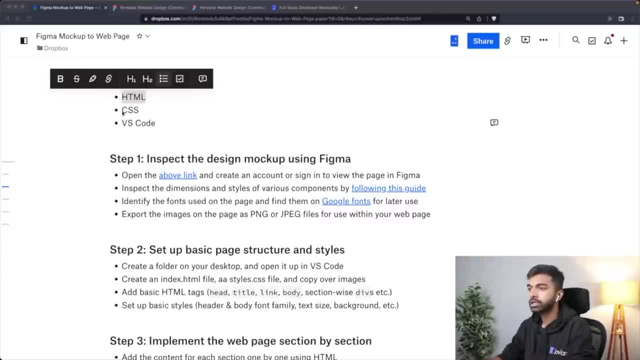 So I'm assuming here that you have some knowledge of HTML. I am assuming here you have some knowledge of CSS, And I'm assuming here you know how to use a code editor like Visual Studio Code. If you don't, then you should check out some beginner-friendly tutorial or come join our 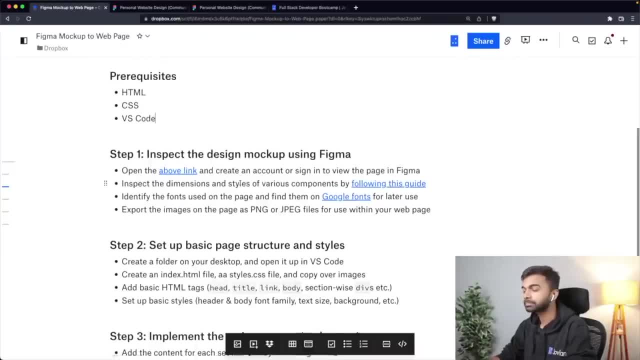 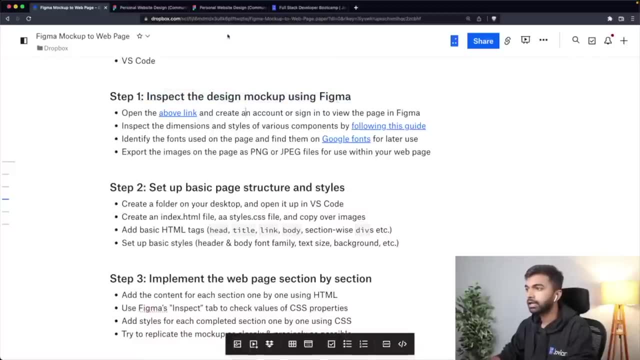 full-stack developer bootcamp where we cover all of these in a lot of detail. Okay, So the first thing is to inspect the design mockup. Now, of course, we've opened up the link and we have created an account on Figma. 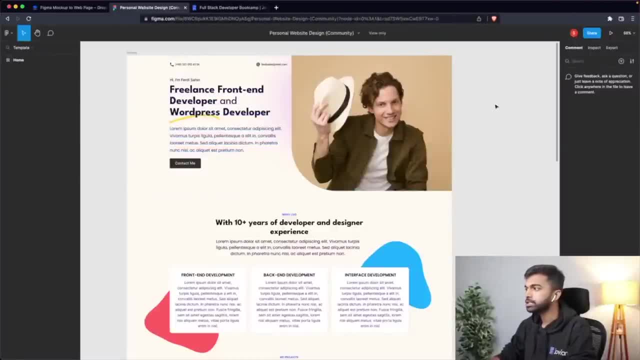 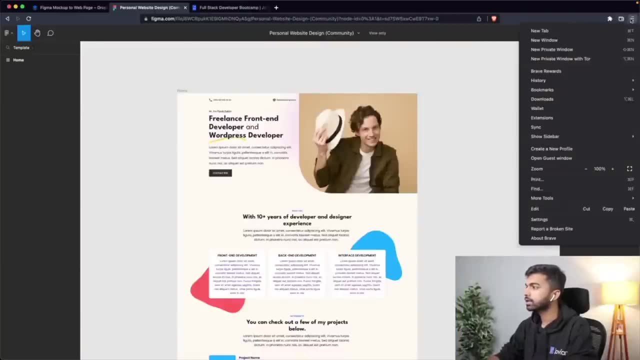 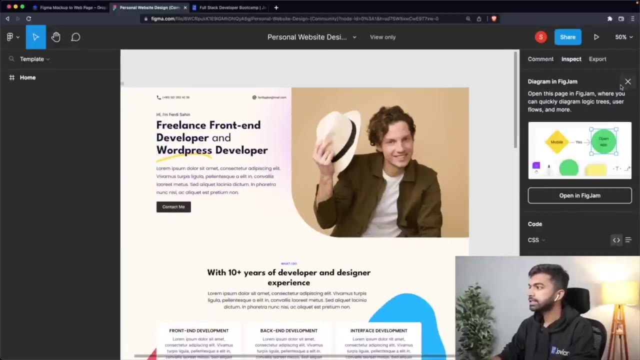 So we can actually inspect the mockup And once you've created an account, you can go into this inspect tab on the right. Okay, So let me just zoom in here a little bit so that you can see things a little better. So, on Figma, you have this inspect tab and this inspect tab gives you a lot of very powerful 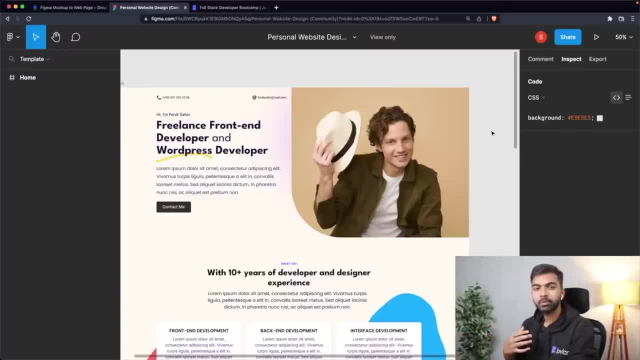 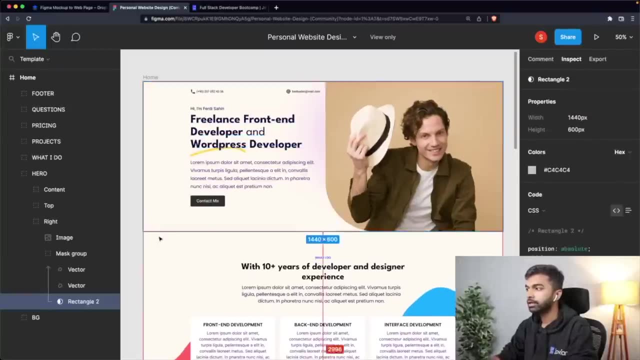 details that you can directly translate into things like CSS properties, colors, fonts, et cetera. So, let's say, I want to check what exactly is the background color here, or maybe the background color for the entire design? Okay, Okay. 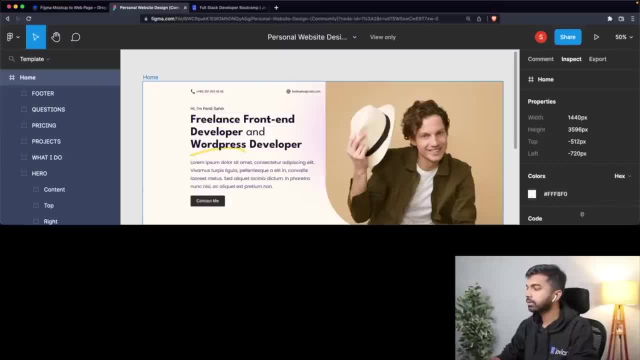 So you can see here that the background color for this entire design seems to be over here: FFF8F0.. All right, So that is how I can pick out the background color, And it seems like this particular design was created with a width of 1440 pixels and a. 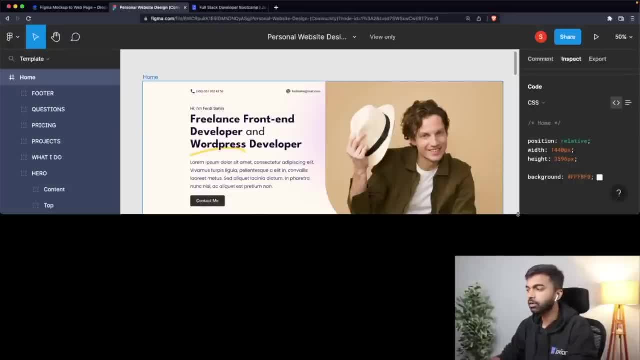 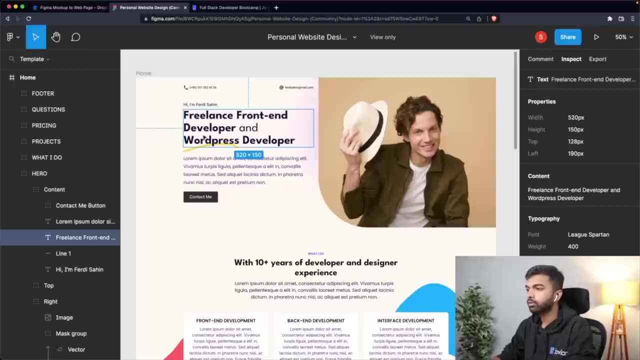 height of 3596 pixels. So 1440 piece is a common width setting that people use. So we're going to use that same width setting and I can go into individual sections. So I can go into this particular section here and here I can see okay. 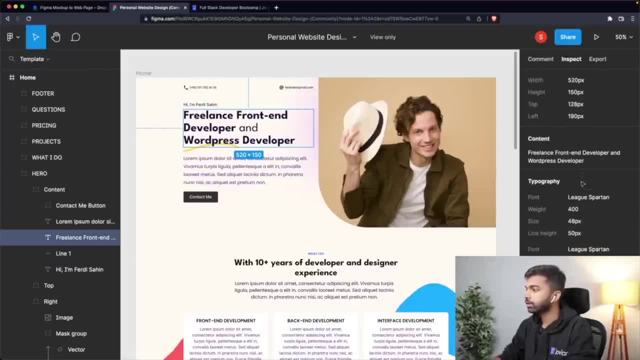 This is the width, height, et cetera. This is the actual text, in case I want to copy the content. This is the typography, So it seems like the font used is league Spartan, and then there is a certain font weight. 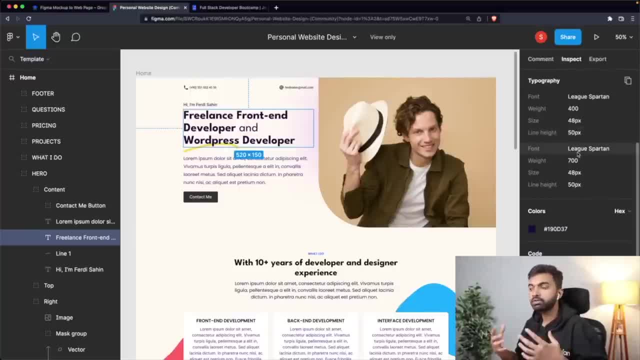 There is a certain font size. So all of this information is going to be useful when you start putting in some of the CSS for our page, And there's a bunch of information about the CSS as well that we'll try and use later. Okay. 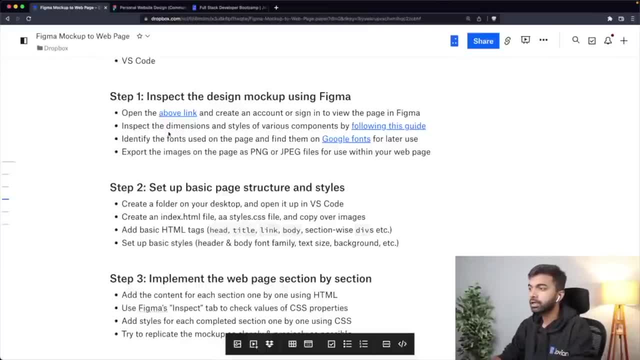 So first thing you should do is just inspect a few things and figure things out, understand the dimensions and styles of weight, There's components- and identify the fonts used on the page so that we can find them on Google fonts. So, for example, the font used here on this page is called league Spartan. 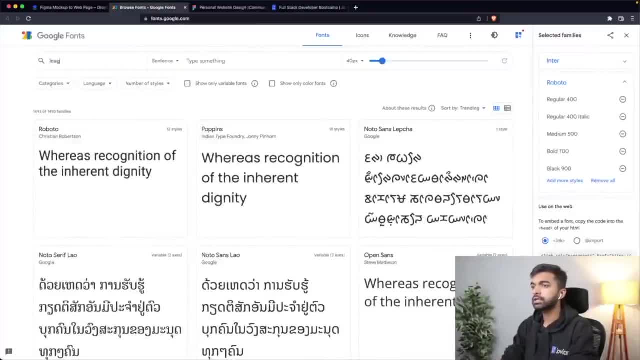 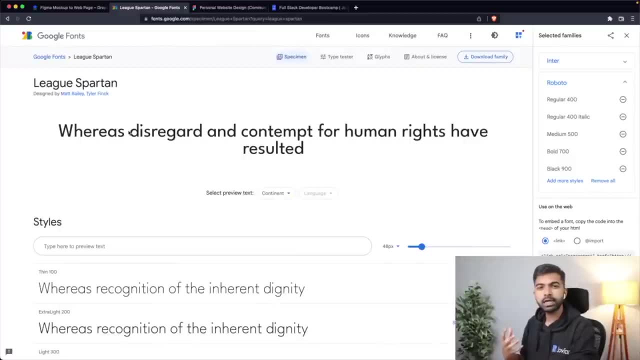 You can see here. so I can just come in into Google fonts and I can search league Spartan and here is that font right. So most fonts that designers use will be picked from Google, will be available on Google fonts. So you will have to then include those fonts within your web page to actually find them. 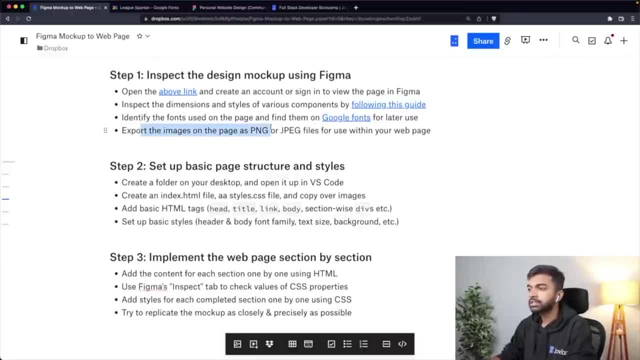 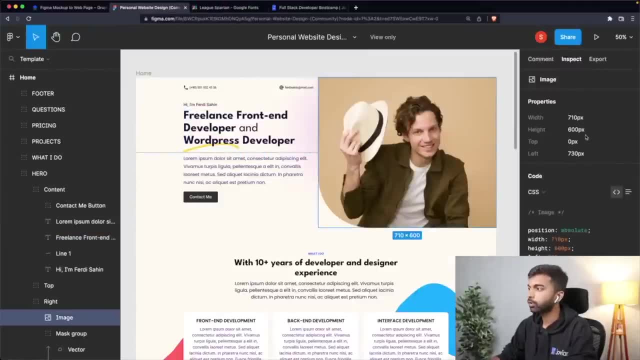 You might also want to export the images as PNG or JPEG files. So here, for example, in this mockup, we have this image and this image may need to be exported. So you can just go to the export tab and you can just press plus and you can export this. 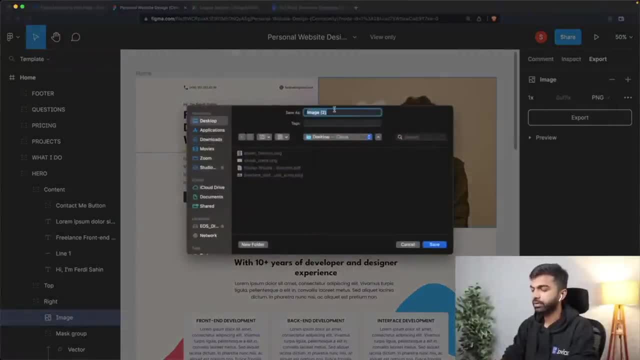 image. So let me just export this image as, let's see, let me just call it hero image. So this is, since this is part of the hero section- the top section is often called the hero section- I'm just going to put it on my desktop and call it hero image. 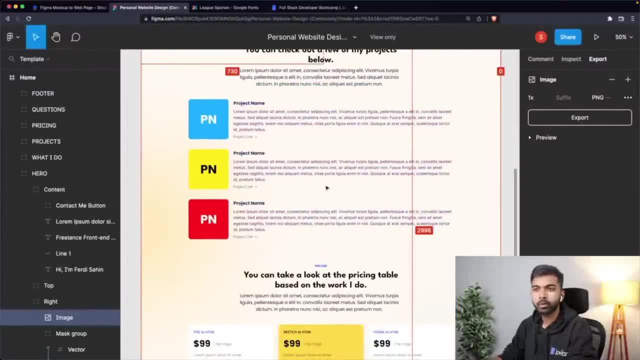 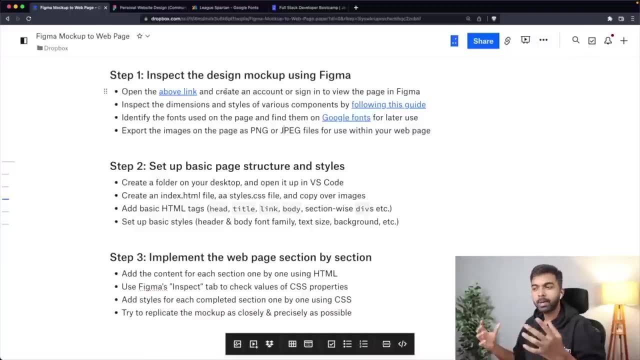 Right, And similarly, if there were other images on the page, you could also export those images. We don't have to do it immediately, We can do it slightly later as well. All right, So that would be step one, inspecting things, but let's now start coding. 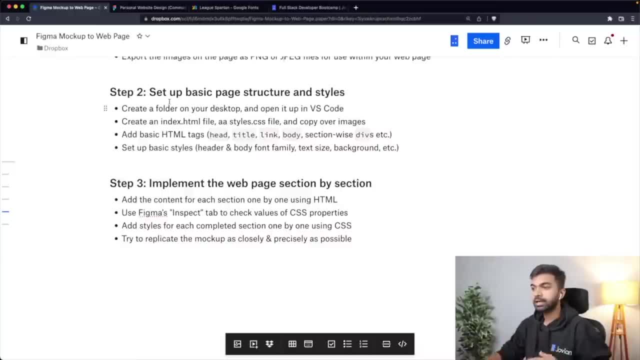 So step two is to set up the basic page structure and styles, and then step three is to actually go ahead and implement the web page section by section. So first I'm just going to create a folder on my desktop and open it up in visual studio. 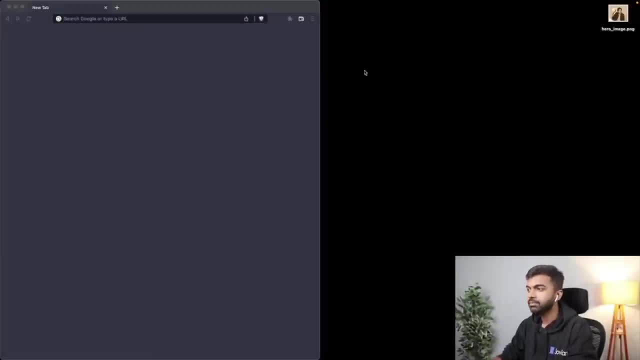 code. I'm not going to use gate or anything here. I'm just simply going to let me see, Let me create a new folder, and let me say, let me call it, Let me give it a name: Figma to web page. 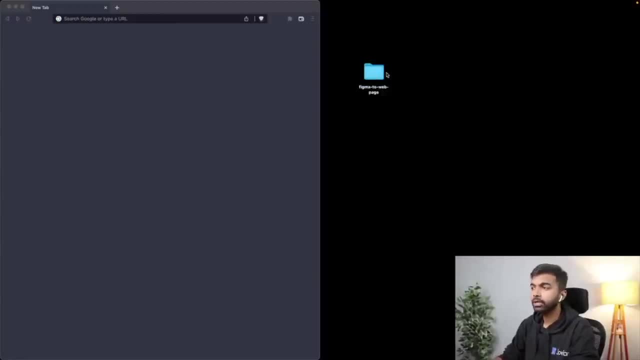 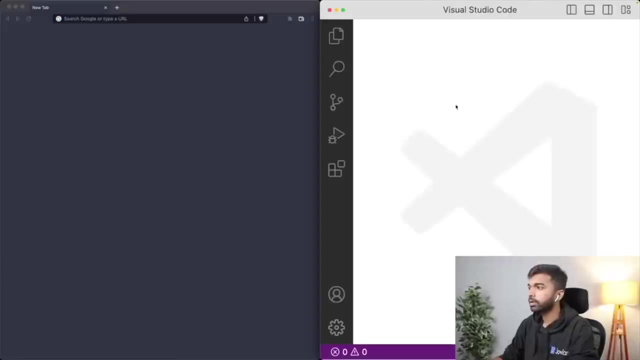 And in this folder I'm also going to move in my hero image that I just downloaded, And I just want to open up this folder in visual studio code. So let me just open up visual studio code. This is the code editor that is often used by web developers. and on visual studio code, 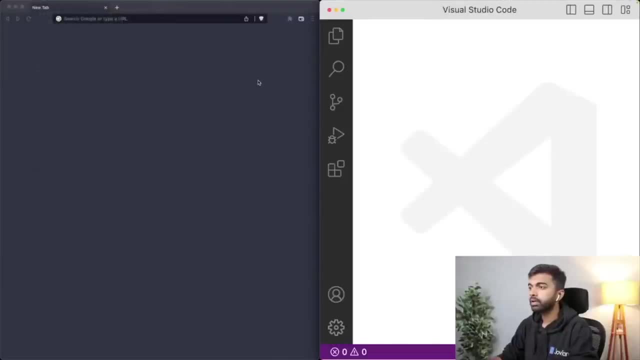 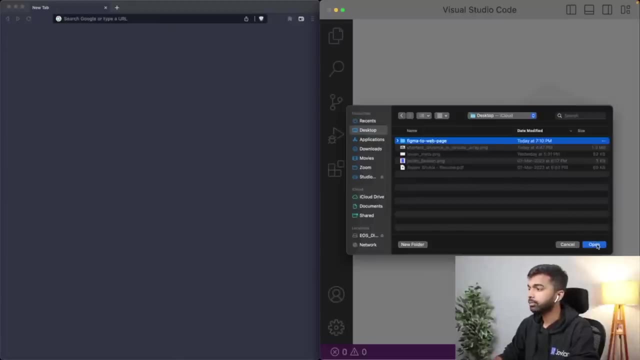 I'm just going to go to file- open folder And I'm going to create a new folder. Okay, So I'm going to navigate to the folder on my desktop: Figma to web page. So here I've selected the folder Figma to web page and I'm going to click open. 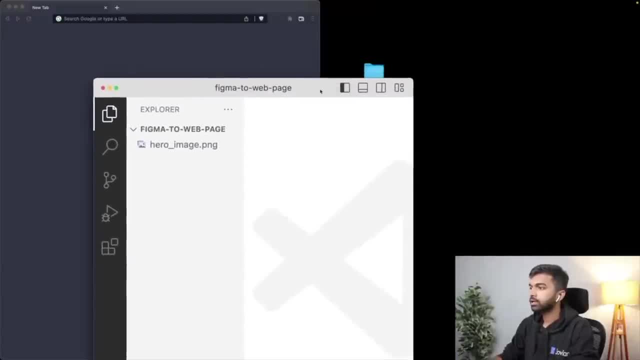 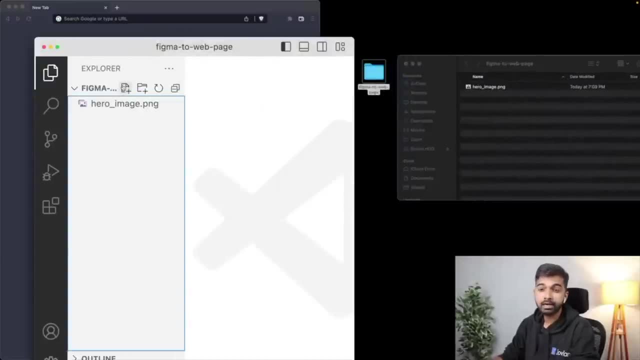 All right. So now we have this folder Figma to web page over here And in this this folder has been opened up in visual studio code and now I can start developing, So I can create a new file and I can call this file index dot. HTML. 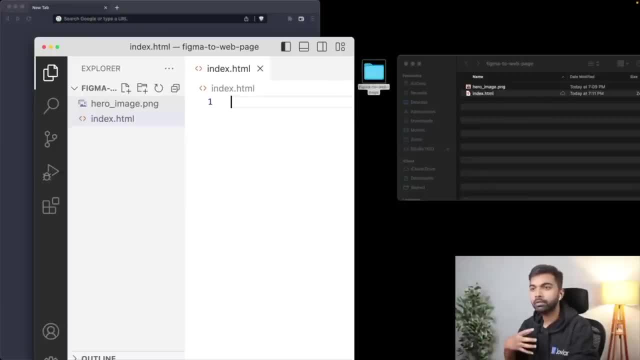 And this is going to be my HTML file, which is going to contain all of the HTML code, And I'll add a CSS file later on as well, And you can see that the same file got added here too, And let us put some very basic content into this file. is index or HTML. 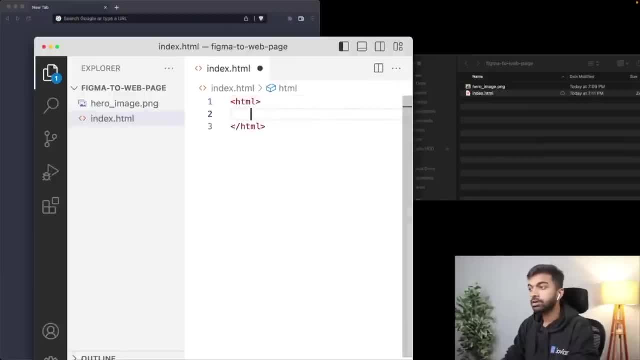 Let us just put the HTML tag again. I'm assuming here you have some knowledge of HTML, but in case you don't take up, a very basic tutorial should be sufficient to follow along with what we're doing here Now. within the HTML tag, we generally have a head tag and a body tag. 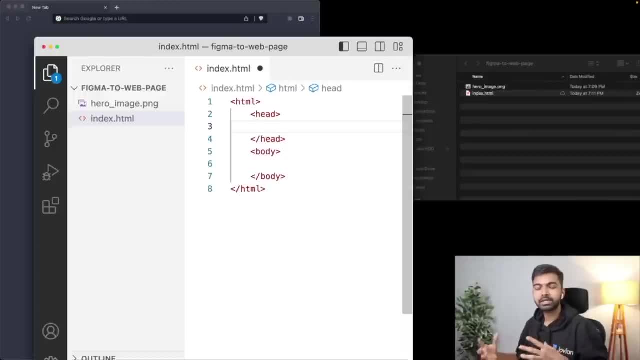 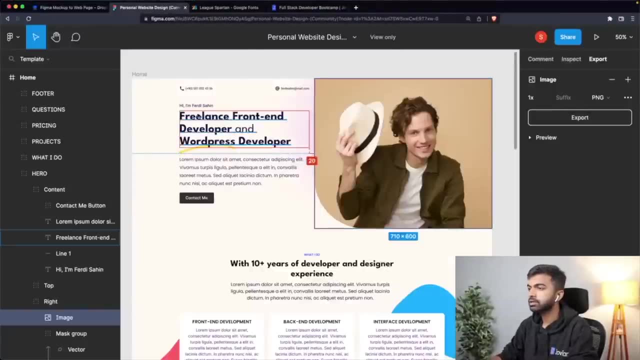 The head tag is where we are going to put all the links like CSS, JavaScript, fonts, et cetera. So let's give this a title here. So let's give this a title. What is this is a personal website for Ferdi Sahin. 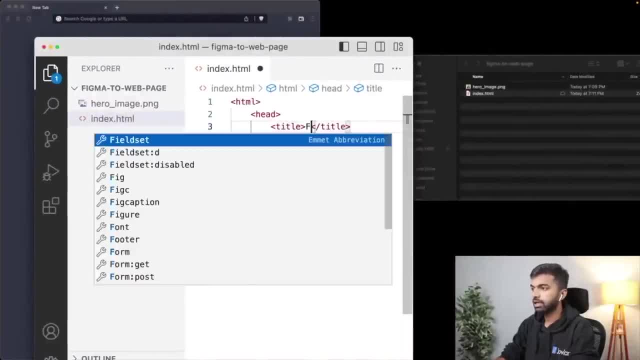 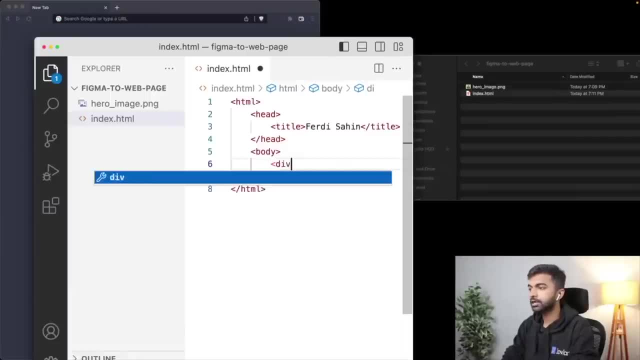 So F E R D I S A H I N, so let's just put F E R D I S A H I N, Ferdi Sahin, and let us in the body. let us, let us just create a div and let us just put hello world here in the 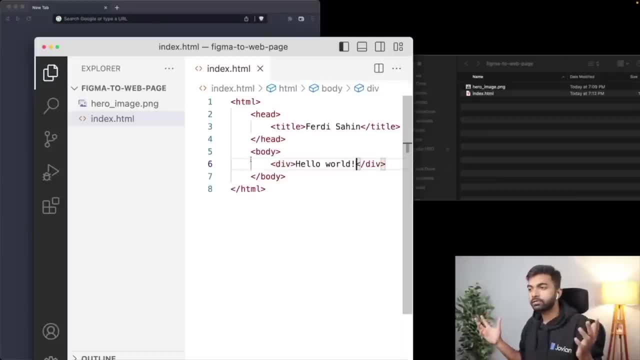 div. Okay, So I've done nothing here, Nothing so far. I've just created a folder. in that folder I've created an indexhtml file, and that indexhtml file Now Has some HTML content, very basic stuff, And now I can open up this indexhtml file in a browser. 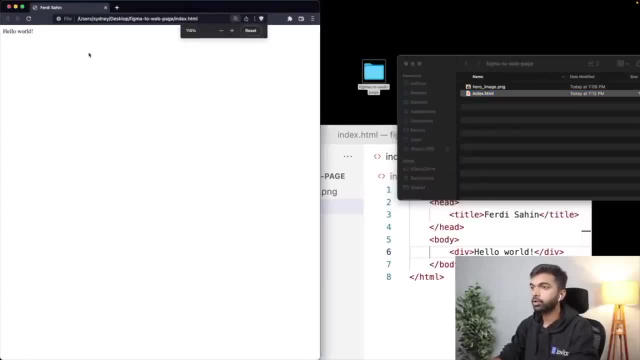 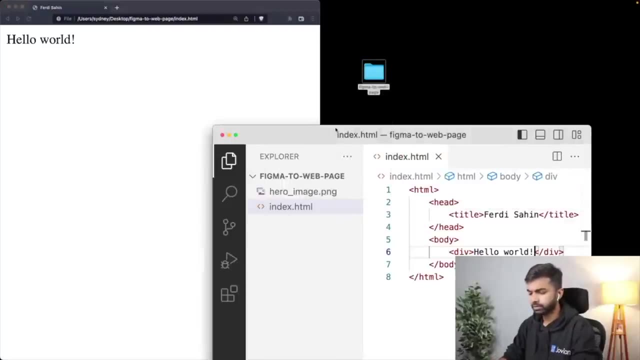 So I can just double click And here you can see that the file has been opened up in a browser over here, If I zoom in a little bit. and now we are ready to get started. So let me just put this on the side and I'm going to close the sidebar for now as well. 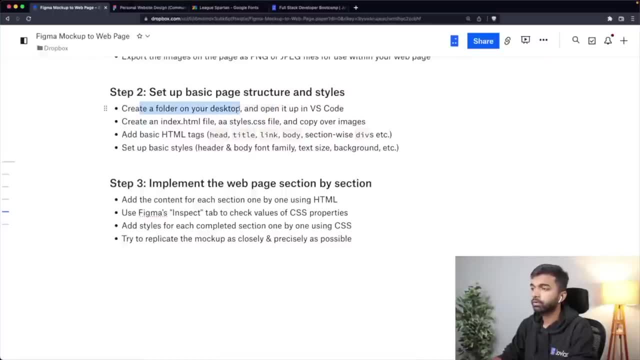 So now we have done the first thing. we've created a folder on our desktop, opened it up in VS code. We are ready to go. Then we are going to create an indexhtml file And we are also going to create a stylescss file. 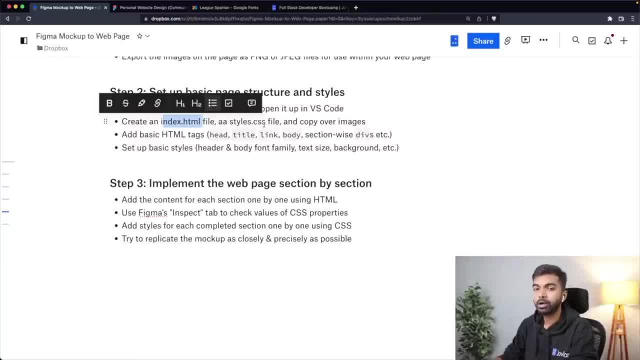 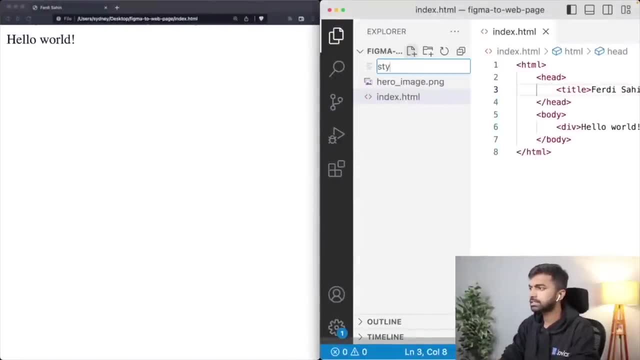 That is something that we will also need to add, where we are going to add all our CSS, and we have copied over the image that we were using here. There's just one image, So let me create another file called stylescss. All right, 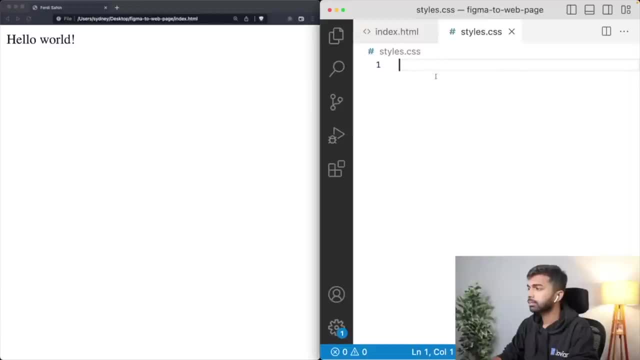 Perfect, I've created a file, stylescss. This is where my text or my CSS is going to go, And now I need to incorporate the stylescss file. I need to link this file from indexhtml So that I can use the styles from this page. 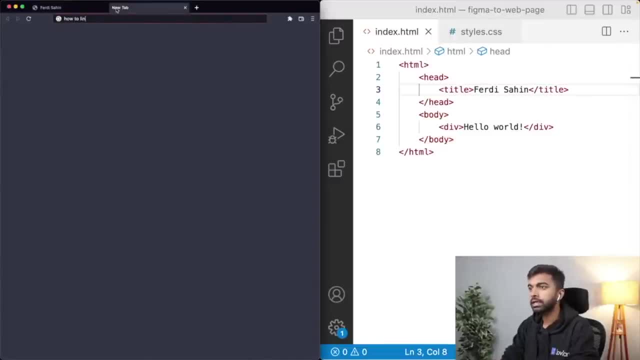 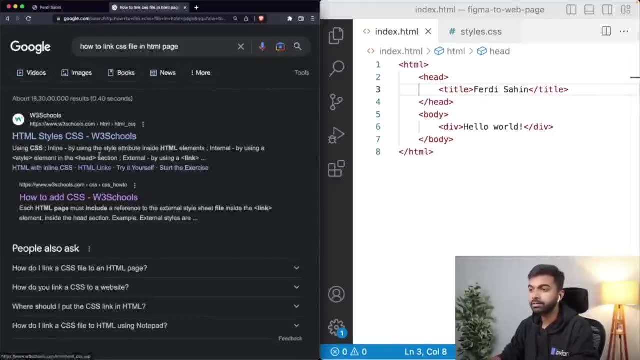 All right, And I'm just going to search. So how to link CSS file in HTML page. I should be knowing this, but I keep forgetting this, So I just look it up. So, HTML style CSS: how to add CSS. All right. 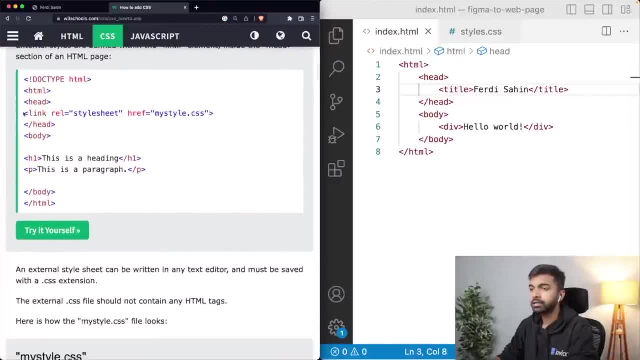 And there are three ways to add CSS. We want to add the external CSS file. So the external CSS file is simply, we simply do this: link rel equal to stylescss And href equals my stylecss, So I'm just going to add that link: rel equal to stylesheet. 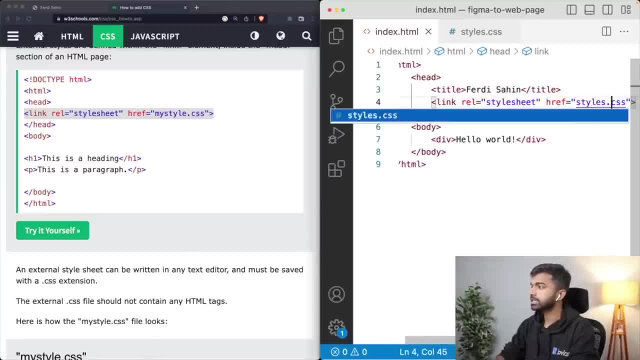 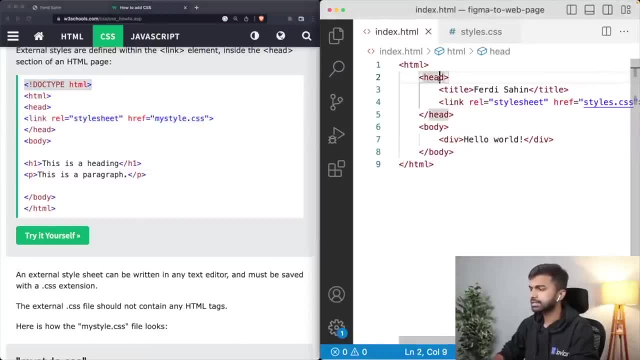 Of course, in this case it's not my stylecss, it is stylescss. That is the CSS file that we are using, And this seems to be this doctype HTML that is there here, So let me just put in this HTML here as well. 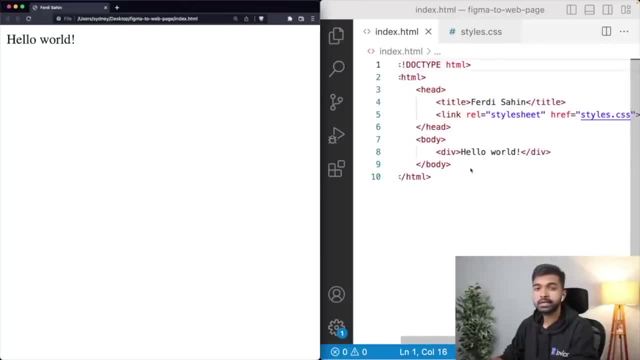 Okay, All right. So now we have set up the indexcss, the HTML file, We have set up the stylescss file and we can verify that things have been set up by, let's say, going into the CSS file and adding some styles. 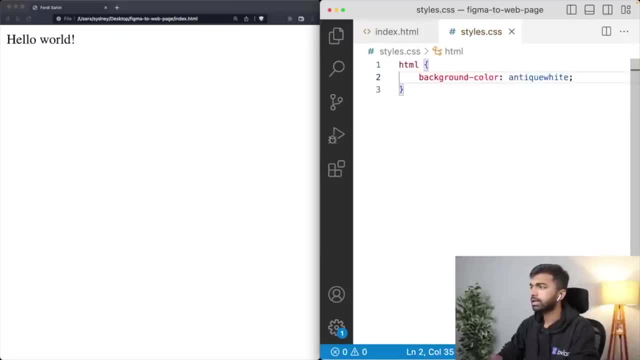 Let's say, let's add a background color- antique white- and let's save it. Let's reload the page and you can see that the color of the page, the background color, has changed. All right, So I'll just reset that for now and get back to where we were. 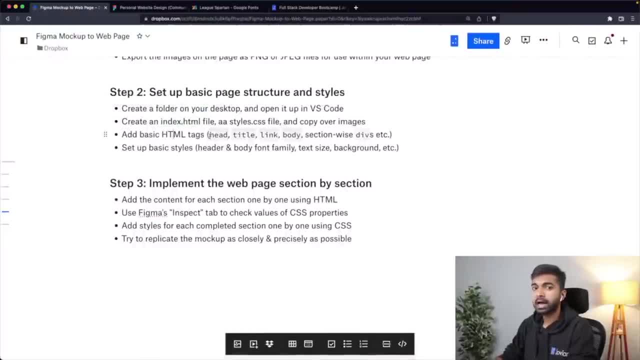 Perfect. So now the next thing for us to do is to add the head title, which we've done already, the link tag for the style and the body And maybe add section wise divs. So we have a bunch of sections here. 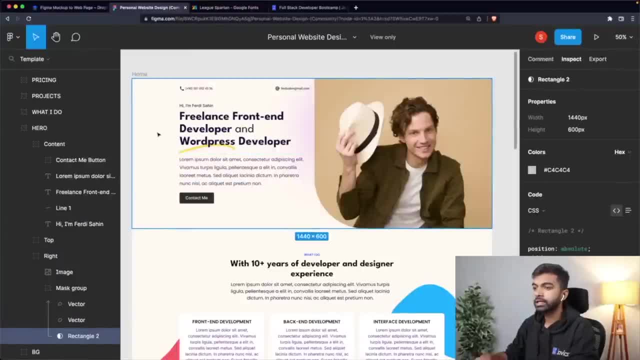 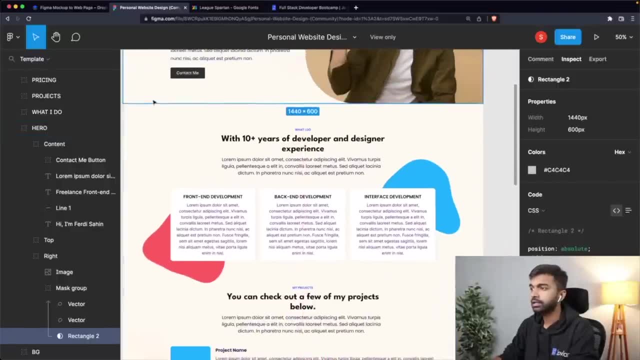 Let me come back here into the design. So I'll call this the hero section And you can see here even the designer has called it the hero section. So this is the hero section. Then under the hero section we have this: what I do, section. 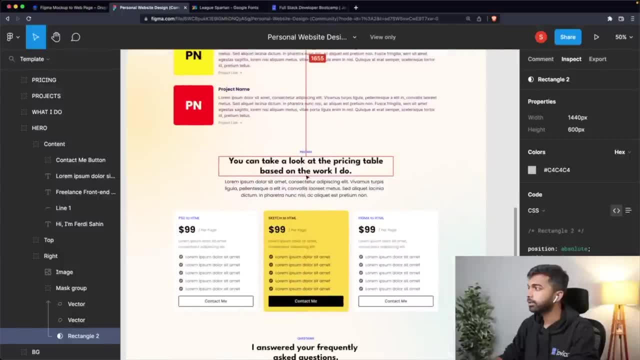 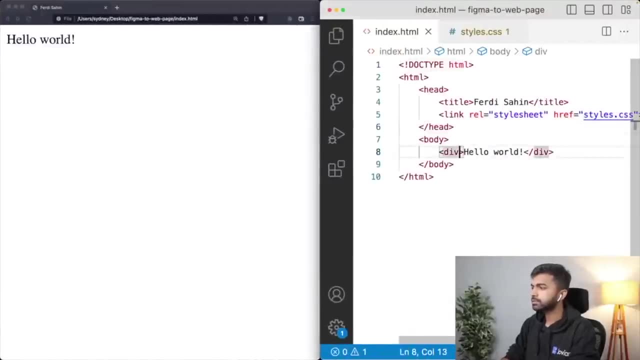 And under the what I do section we have this project section and under under the project section we have this pricing section and the question section. All right, So let's just create a bunch of divs. So we have a top level div called hero. 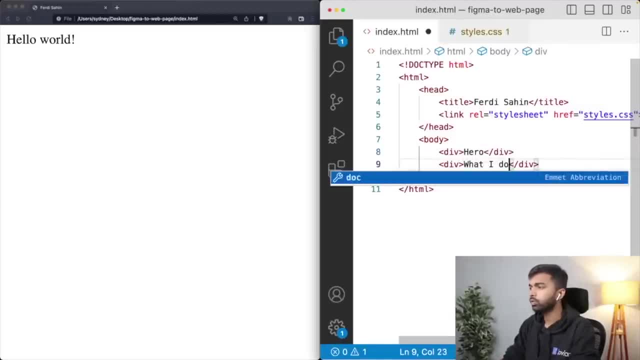 Then let's create another div called what I do, And then let us create another div called projects, Then let us create another div called pricing, Let us create another div called questions and let us create another div called footer. There's also that black footer at the end. 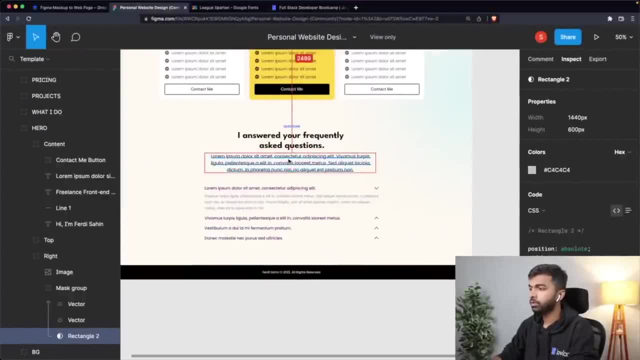 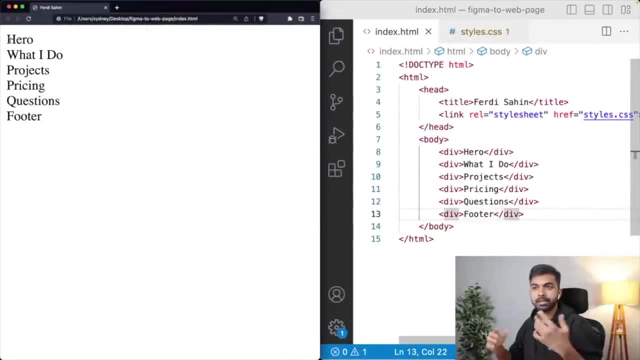 So I am going to have another thing for that as well. So one, two, three, four, five and six. So we have six sections and let's reload that. And this is we are. this is what we're hoping is going to eventually turn into the actual 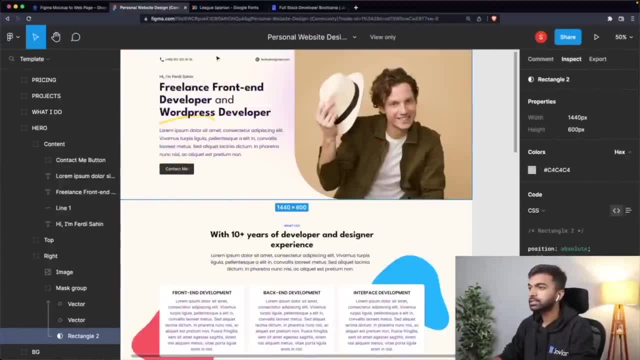 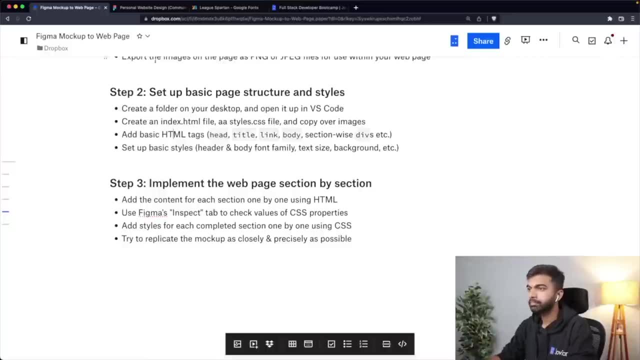 web design, the page that we are looking at. Okay, Perfect, So now we've created these sections, What next? set of the basic styles: header, body font, family text size, et cetera. So let's start setting up some of the basic styles here. 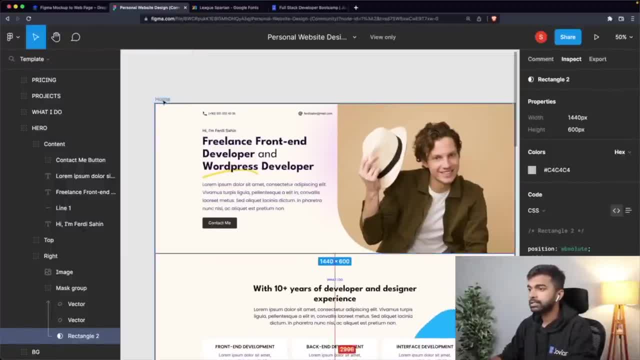 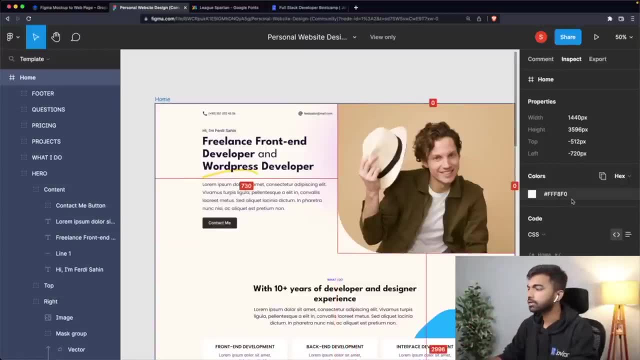 Okay, First thing. first is the background of the entire page, So I'm just going to go in, I'm going to select the entire. this is called a frame in Figma, So I can just click on the frame name and get the frame and looks like this is the color. 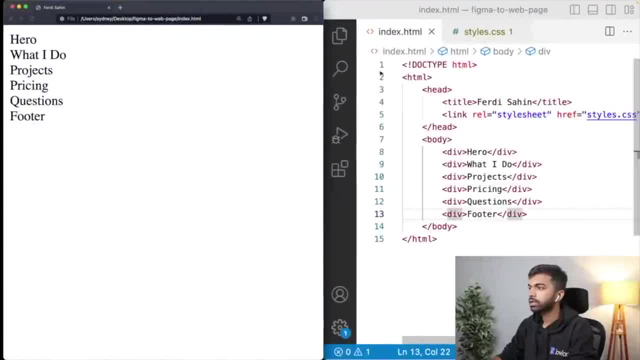 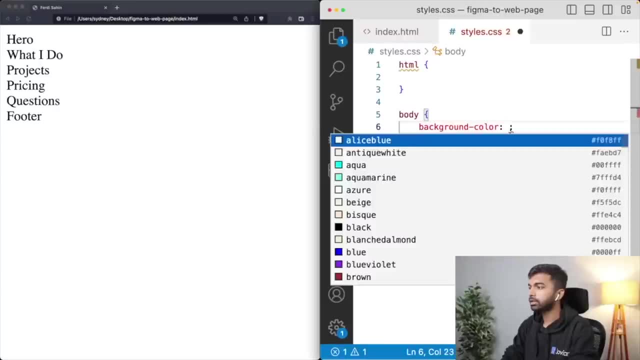 that is being used here. So I'm going to go in here and I am going to come into styles, dot, CSS, And for the body, I'm going to set background color to this color. Oh, okay, I think I didn't need to type. 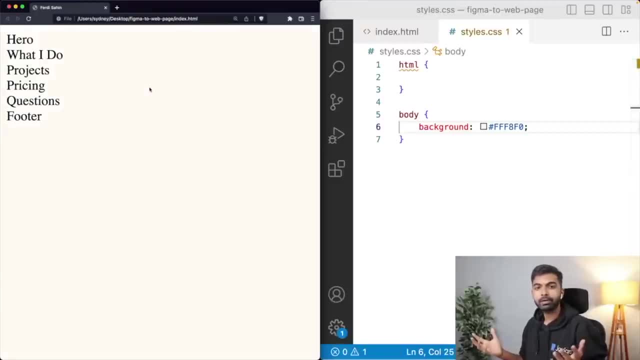 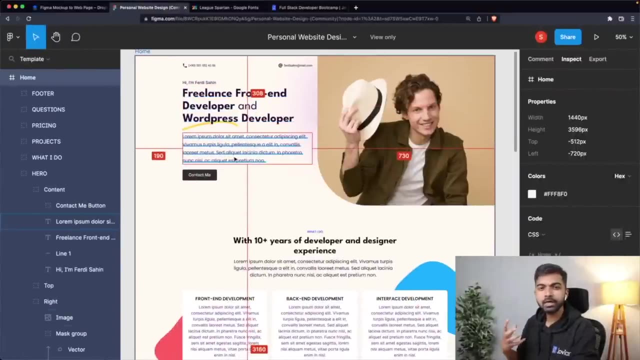 Yeah, So background is this color, And now we've added the background, So we're starting to make progress. We've added the background. Step one is done. What next? So I might need to just study the fonts that are used on the page and include those fonts. 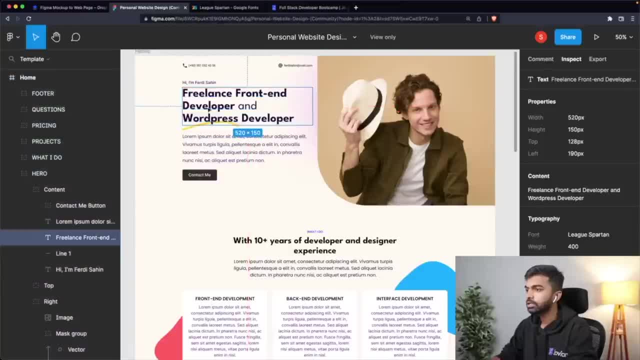 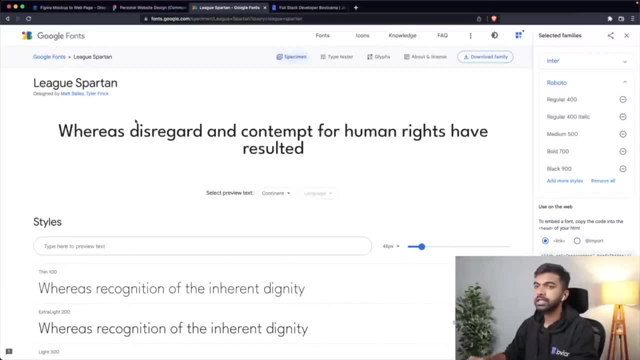 from Google fonts into my project. So here is one font. There is this one called league Spartan that seems to be used here. So league Spartan. Okay, I want to use the league Spartan font and I found it on Google fonts. So let me just seems like I have some selections here already. 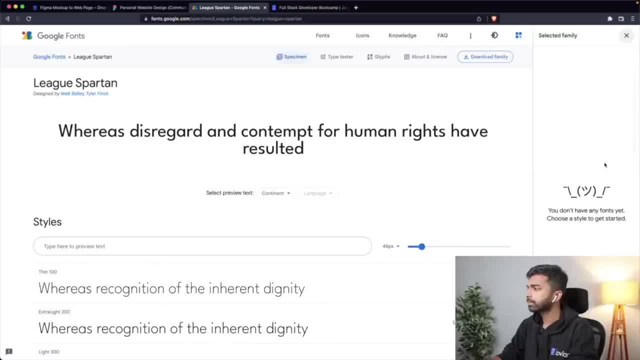 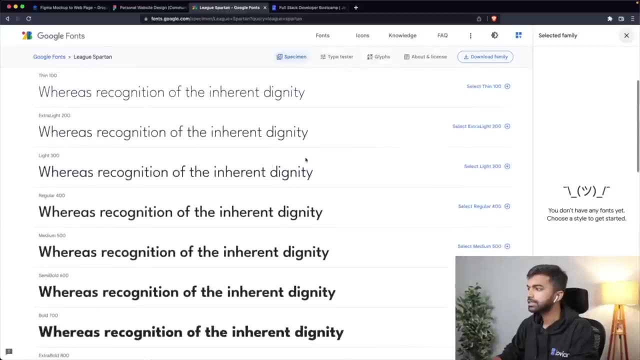 Let me get rid of all these selections so that I can go ahead and do this from scratch. Okay, So the league Spartan is the font I want to use, and let's see, let's get all the weights and we will get rid of some of the additional weights. 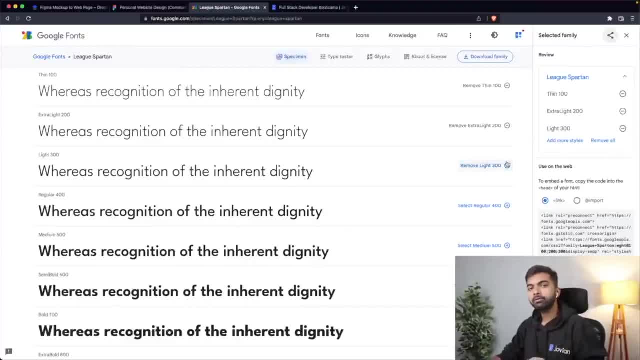 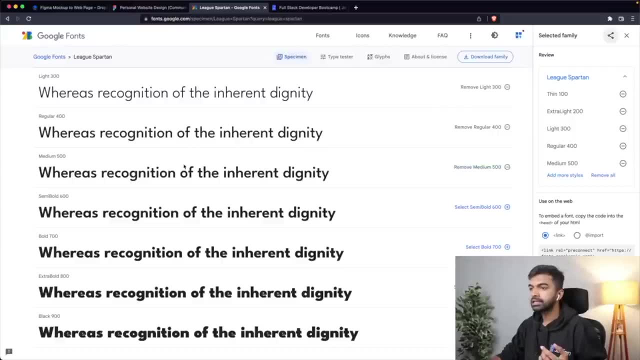 So Google fonts is a place where you can find all kinds of fonts and to incorporate a font into your website You can just add a bunch of styles of the font so you can see that there are various font weights. There's a thin font. 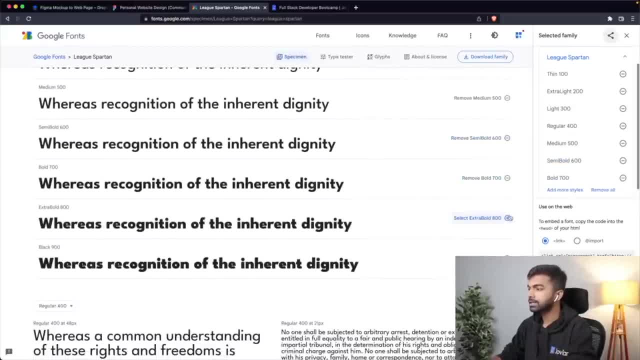 There's a thick font, regular font, and also I'm just grabbing all of these so that I might need to use any of them. I'm not sure I'm grabbing all. I'm just going to go in and edit the, the link tag or whatever I incorporate so that 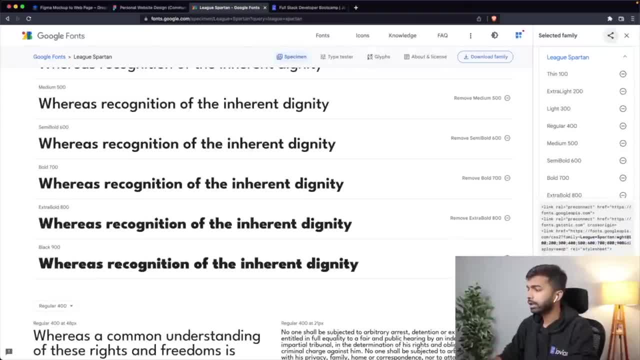 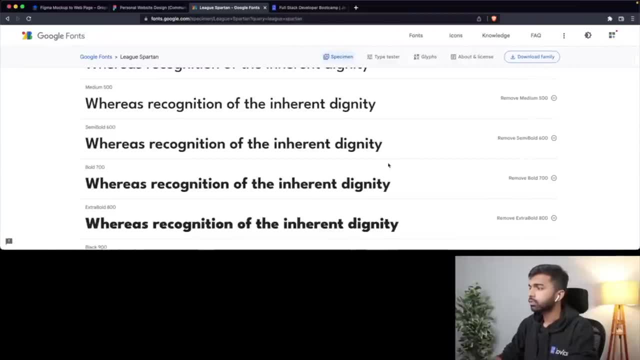 I don't. I don't have to worry about including additional fonts that I'm not using, but just to give you an idea of what you're going to get, here is, let's say, close this. So once you add a bunch of fonts, you can see this view. selected families button on. 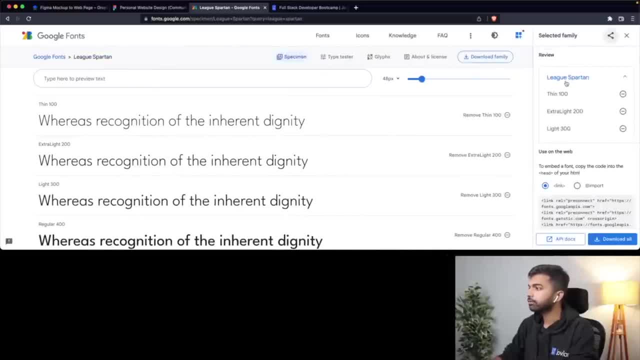 the top right And from there you can check, you can review that. Okay, For league Spartan, you have selected a bunch of these fonts and then to use that font on your website You can then use a link tag. So to use the link tag, you simply copy all of these and then you go and add that within. 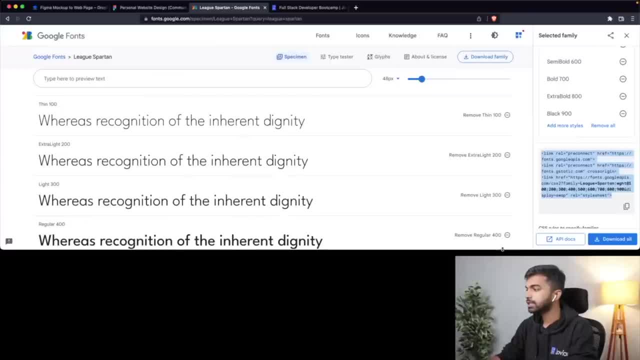 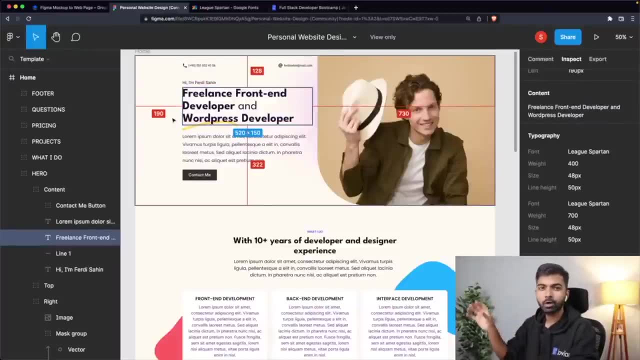 the head tag of your HTML page. But of course, league Spartan is not the only font. There are other fonts here as well, So let me go and check what other fonts are being used, so that I can just incorporate all of them into my website at once. 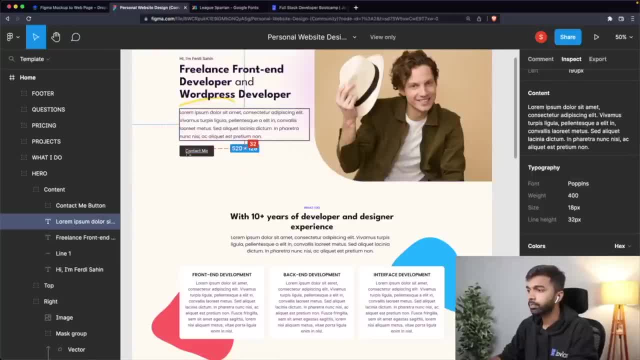 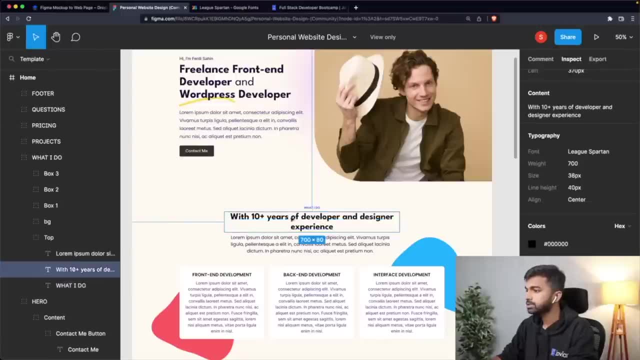 Okay, Now this font over here seems to be Poppins, So Poppins seems to be a font that is used here. and there is this font, inter, that seems to be used here as well. Okay, So this seems to be Poppins. This seems to be league Spartan. 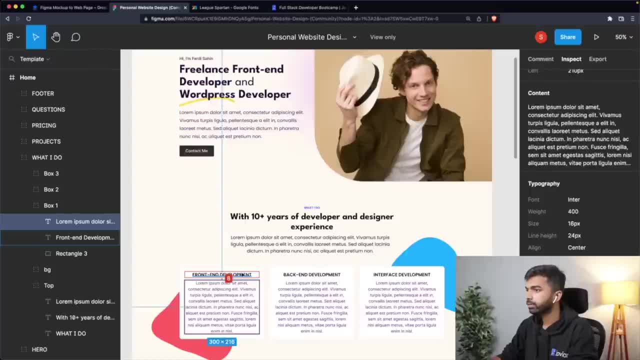 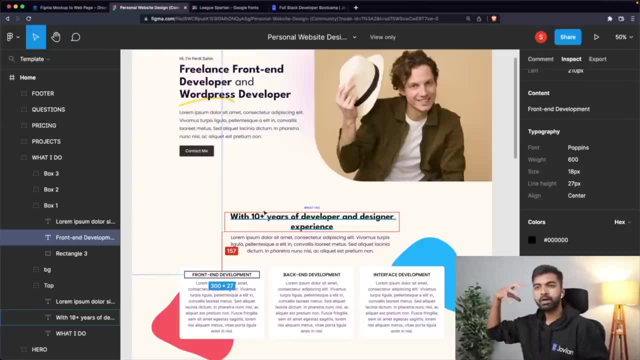 This seems to be Poppins, This seems to be inter and Poppins. Okay, So from what I'm gathering here, there seem to be three fonts here. One is the font that is used for very big, large headings. Then second is the font that is being used for these smaller headings or section headings. 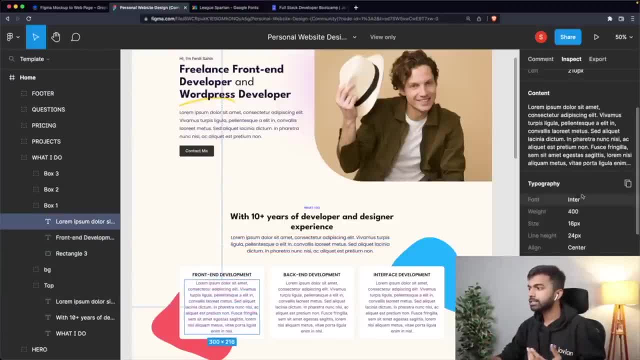 or big text, And then third is the body text, the actual body text, and that seems to be inter. So let me grab Poppins and let me grab inter. Okay, And then we'll, then we'll add all these fonts into our webpage. 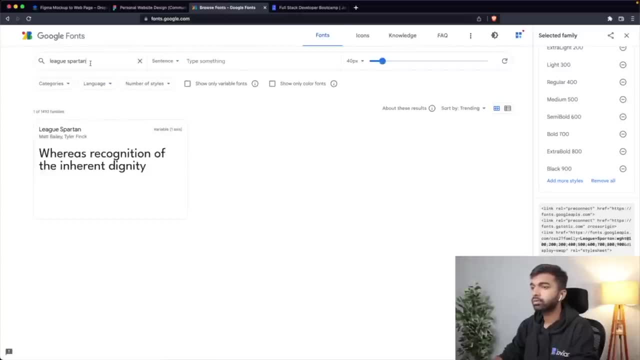 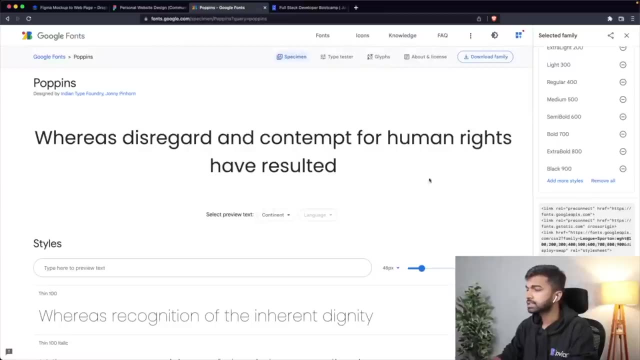 So let me search for the font Poppins. So let's go back to Google fonts. Let's go Poppins. Okay, That is the Poppins font. I am just going to select all the variations right now. Probably not the best idea. 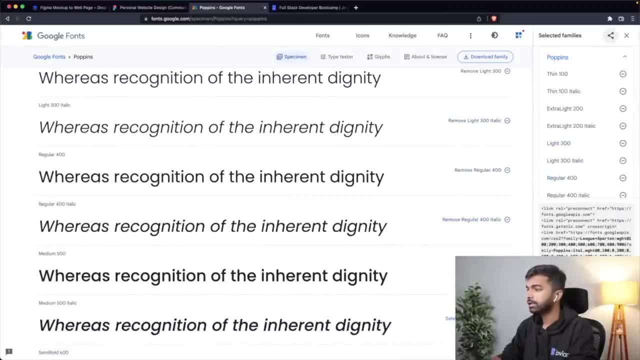 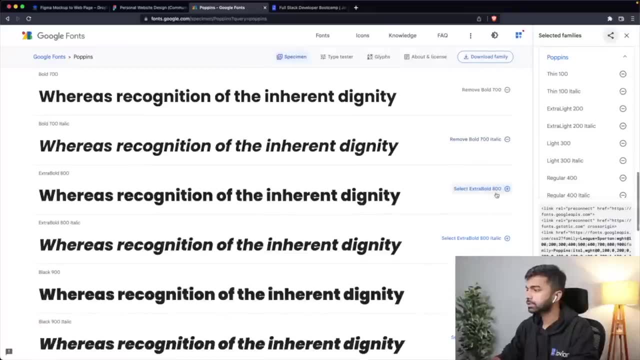 I should probably check with the designer, which all we need to use. but it's okay, We'll go and fix this later. Okay, I am. I selected a bunch of these fonts, All right, Looks like there's a lot of these. 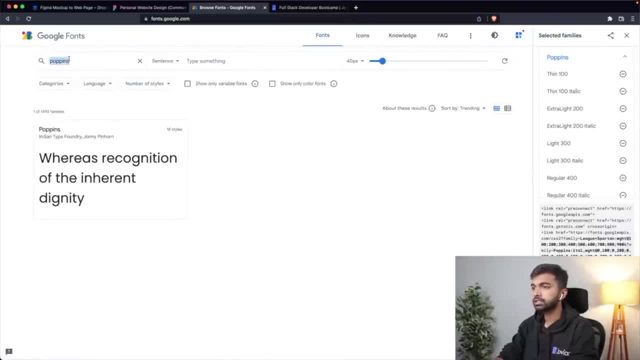 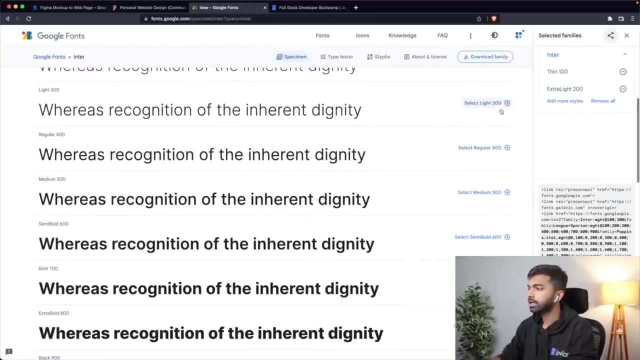 So I've added the Poppins font. Let me go back in, Let me search for the inter font, and I'm going to get a bunch of variations of the inter font as well. Again, I'll just select all of them, just so that we don't have to worry about missing. 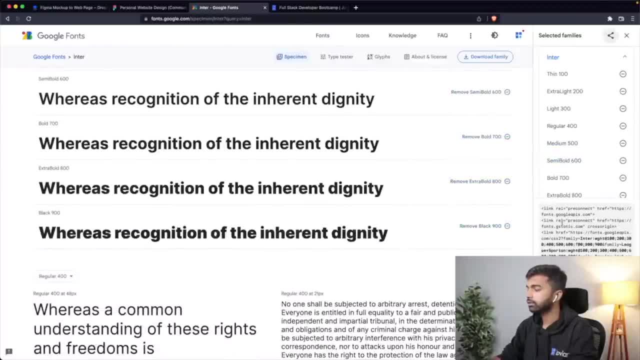 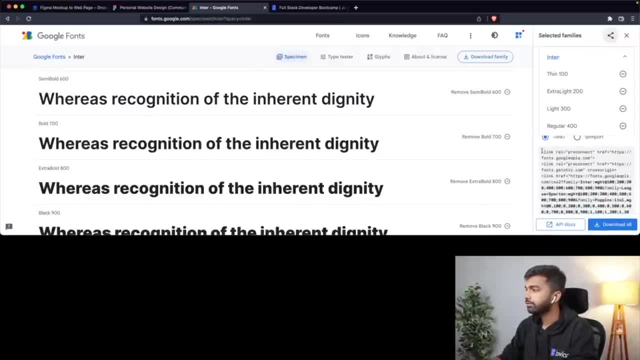 any important fonts. Looks like we got the inter font as well. Okay, Great. So now you can see that our link tag has been populated over here, So we have this link rel preconnected, Et cetera, et cetera. 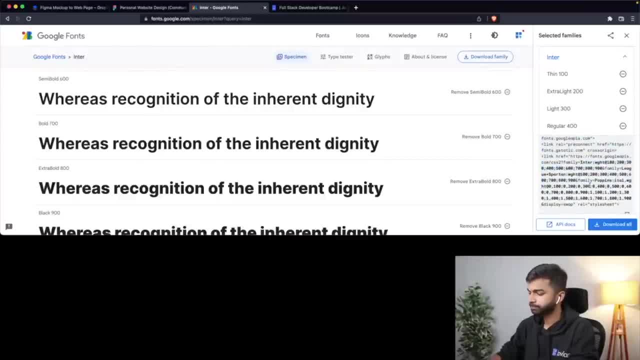 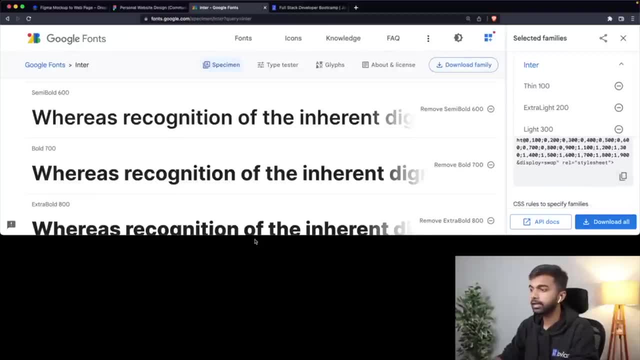 And over here. this is the specific area where we have names of fonts. I can zoom in a little bit. You can see that we have names of fonts and then weights of those fonts as well. So let's just copy that entire link tag. 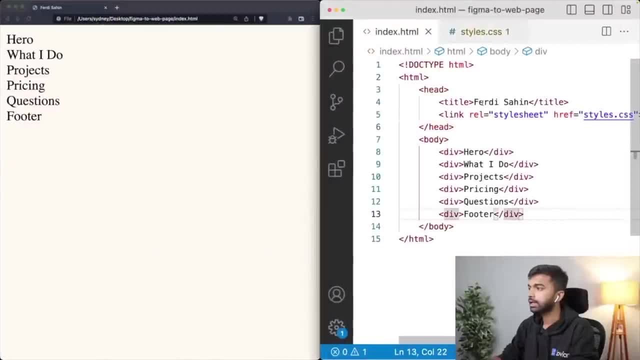 And let's go in and put that link tag into our head. So I'm just pasting the link tag here and I'll just right click select format document so that it just shows up a little nicely. And now we have incorporated all the fonts. 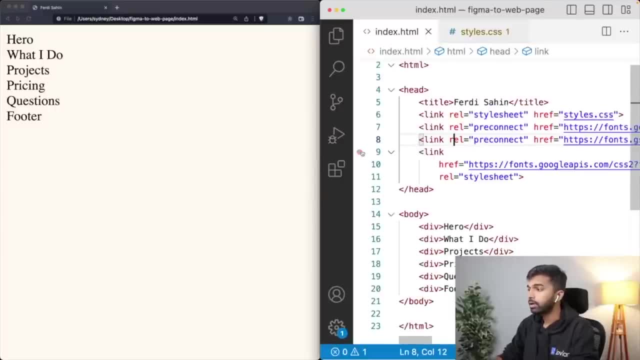 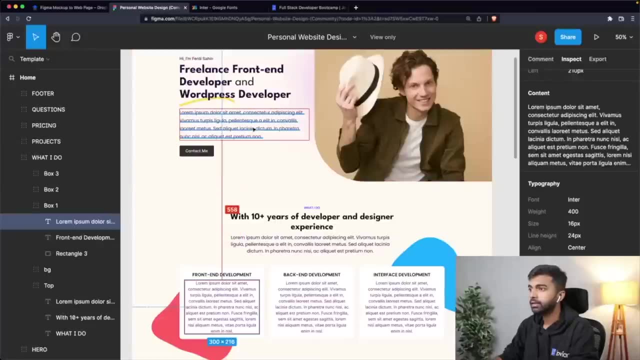 Into our page too. Of course, we've not started using them, We've just incorporated them, So no change happens on the page itself. but let's come back here into the page and let's see. So we have. it looks like inter is the main body font. 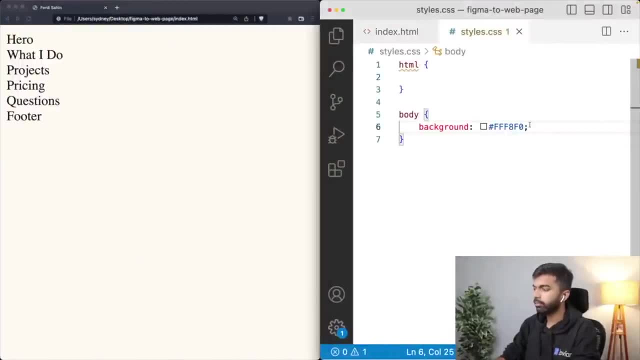 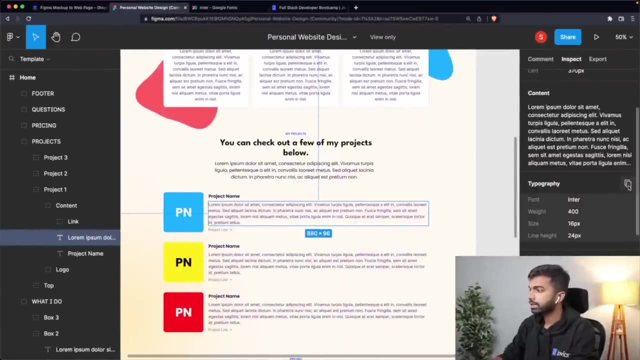 So I'm just going to come in here into stylescss and into the body I'm going to add font family inter. Um, actually, I can just copy this from: yeah, I can just copy this from Figma itself. I can just click the copy button. 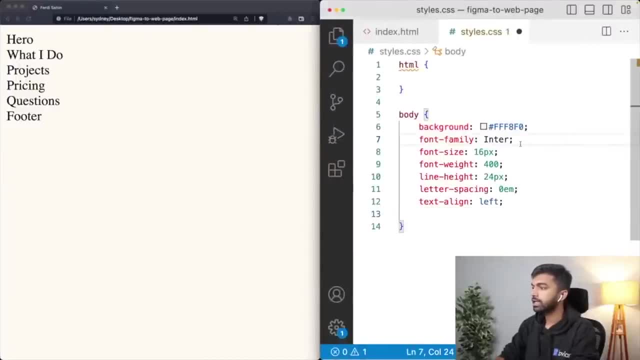 And that's going to copy all of these things. So font family inter the base font size. I'm going to just set it on HTML just so that we can use EMS for relative font sizes. font weight of four or font weight of 400 on inter. 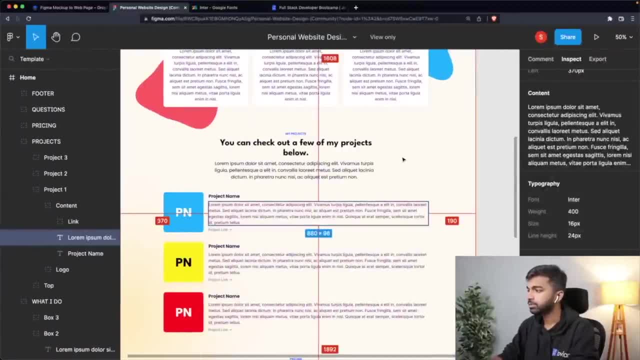 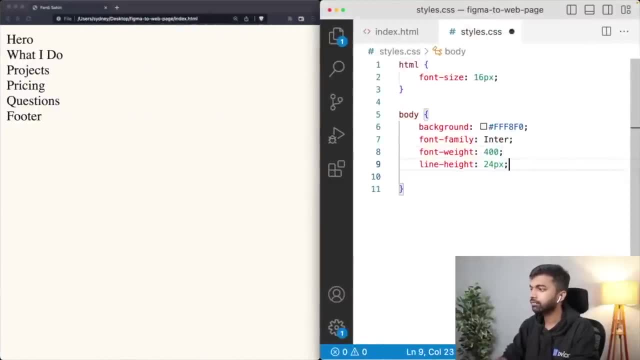 Okay, Then the font line height seems to be 24 pixels. later, spacing: We probably don't need that. It's by default, It's, I believe it's a zero, and then text align left. We don't need that. Okay. So once I do that, I've changed the body fonts and you can already start to see that now. 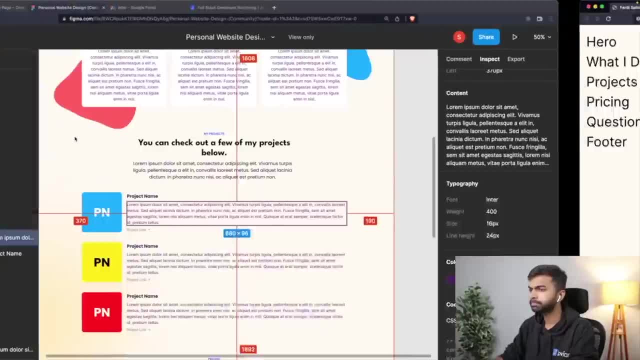 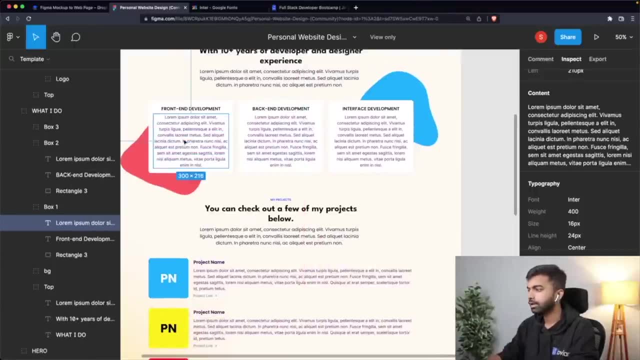 we are getting something that is closer to what we expect. Okay, What about the color of the body text? So the body tech seems to have this slightly- uh, slightly- different color, And this is the color that they're using here. So the color of the body text is 55206D. 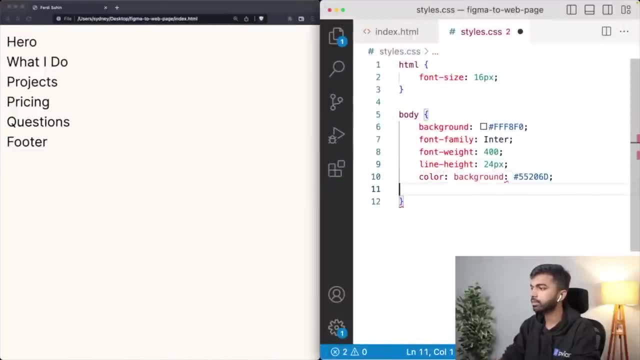 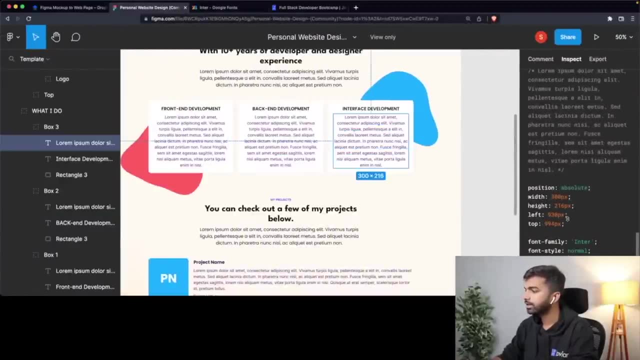 So I'm going to come in here and set the body color, body text color. Let's come back here. Let's see Body text color. It's all added here. So over here we have this color: 55206D. 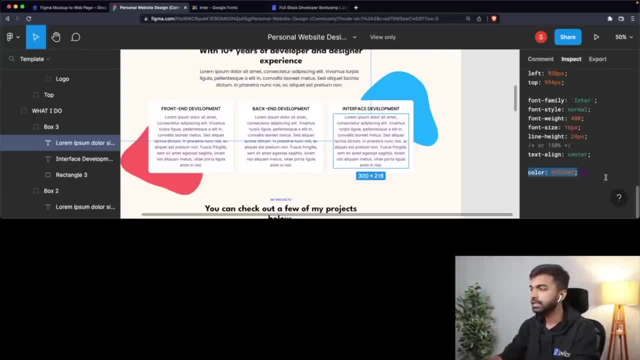 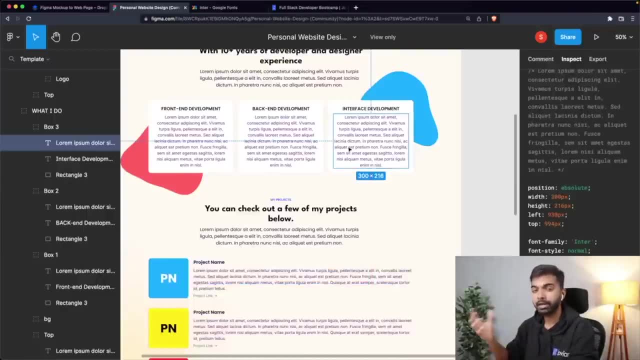 So this is a nice thing about Figma: It gives you the CSS properties that you can use directly. Of course, sometimes the CSS properties may not have an exact mapping. You may still have to modify things a little bit, depending on how the designer has set. 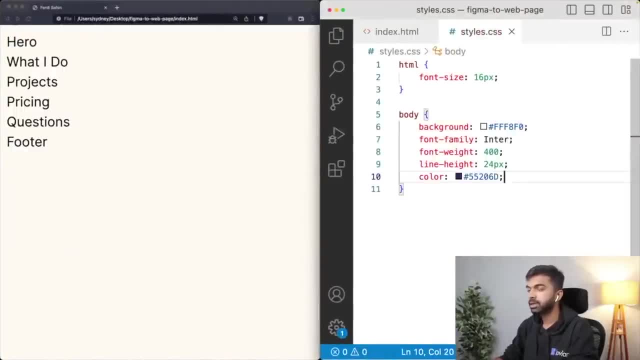 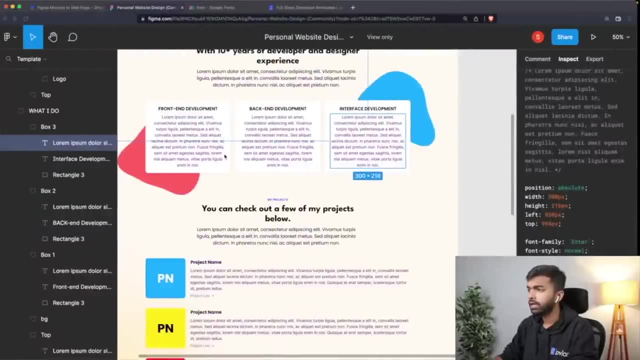 things up, But in most cases you should probably just be able to copy things over. And now you can see that the color of the text has also changed. Great, What next? What next? Well, uh, let us set up, maybe. 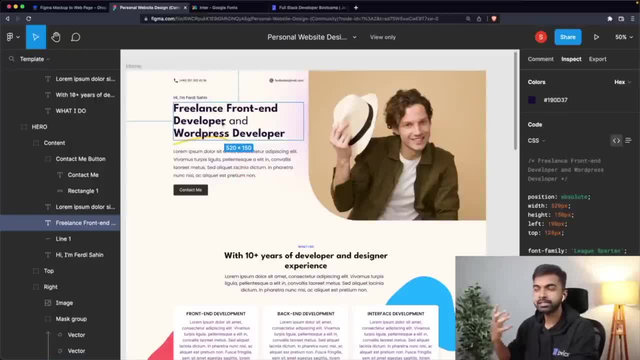 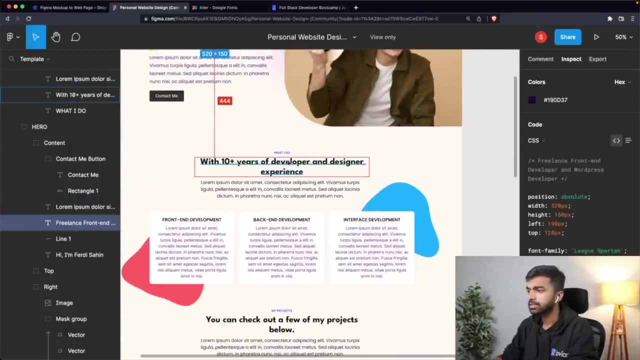 So this is like a heading, This is an H1. There's an H1 tag. So for all the headings- H1 to H6, I feel like, or maybe at least, this is an H1 and then this is an H2 and looks like H1 and H2 are the only headings used. 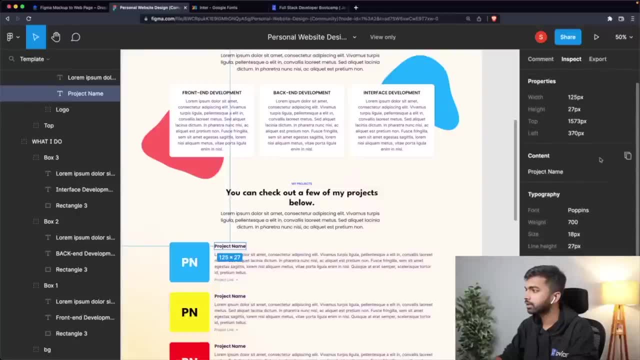 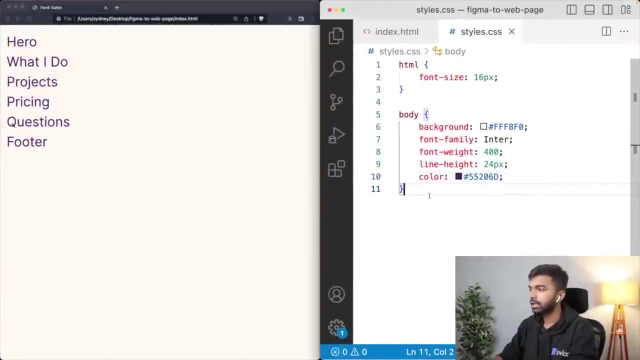 And then this is an H3, which also seems to have the font pop-ins. So for H1 and H2 seems like we're using league Spartan, So I'm going to come in and I'm going to say H1 comma, H2.. 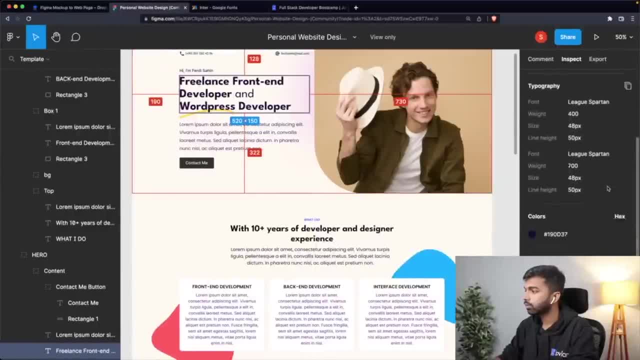 I want to use the font family league Spartan. So let's see font: family league Spartan. So I can just copy that over here. but I can just copy all the typography at once, So let me copy the typography here for the entire thing. 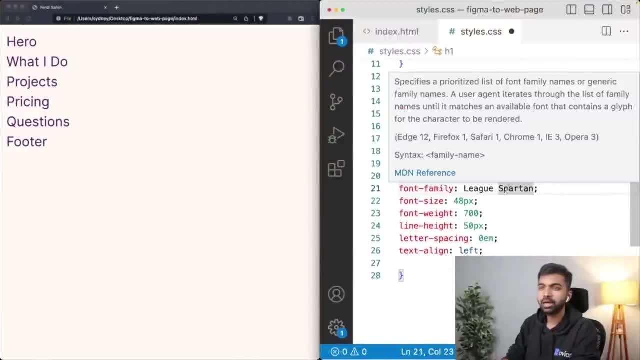 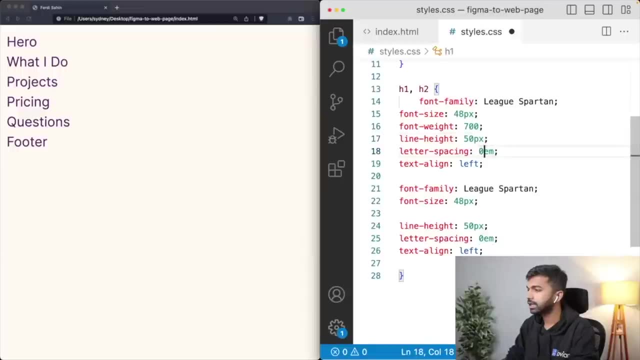 And let me come in here and let me paste it. Of course, sometimes we may have to edit what we paste. So H1, H2.. Let me just put font weight 700.. I'll verify if this is correct. Actually, let's just do H1 for now. we'll do H2 later. 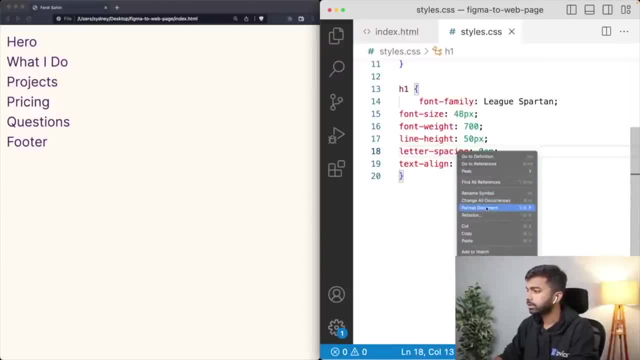 Okay, Let's format this document, And all right. So now for H1, which is the heading of the page, we have set up the font family. We don't need the letter spacing in text line. I think that should be fine. 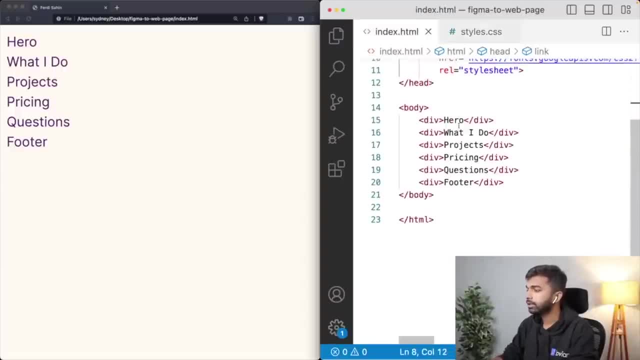 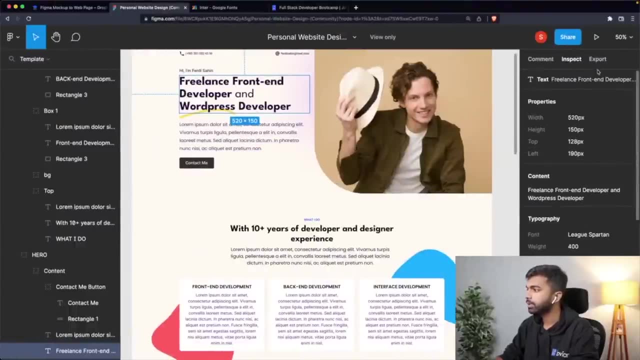 We've set up the font weight, We've set up the line height. so I can come back in here and then maybe I can actually just put in this text directly. So again, I can click on this text, I can scroll down in or scroll up and copy the actual content. 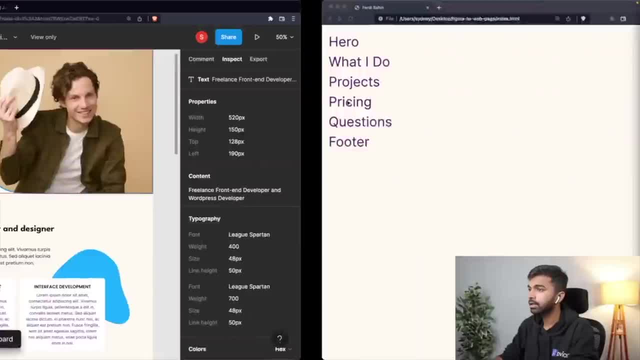 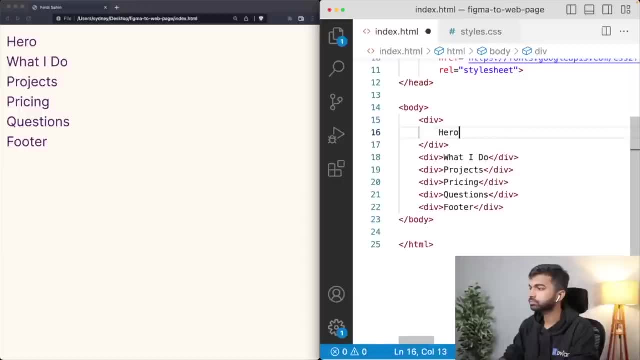 So just click golden, go into the content tab and click copy. Come back here and maybe in the hero section let us just put in an H1 here. So let's do hero section and let us just put in H1 and let's paste this. 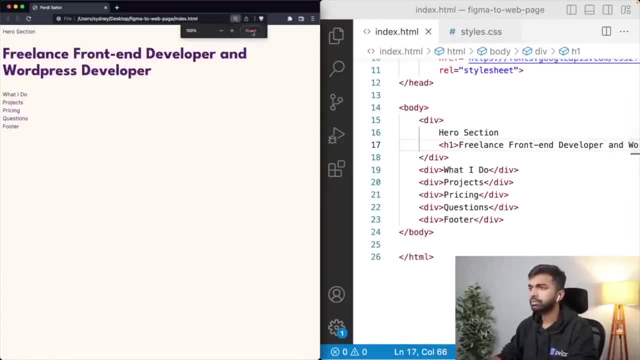 Okay, All right And Okay. So I was using a very big font earlier. That's why I zoomed in version, That's why it was so big. But now that we have this H1 at a big size, I'm zooming, zooming back to a hundred percent. 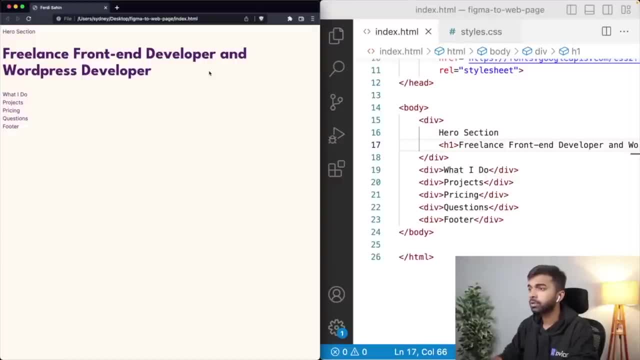 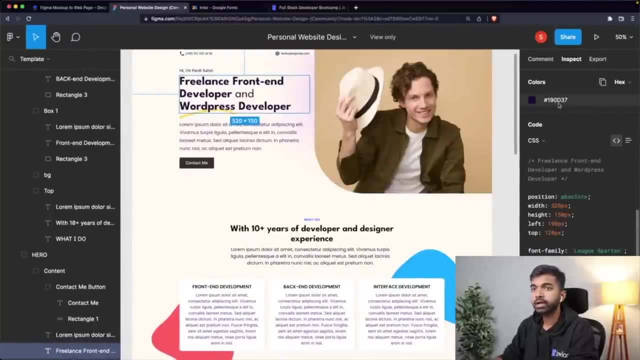 visibility. Okay, All right, So now we have the H1, but the color seems to be off. Like you see here, the color for this H1 seems to be different, So let's grab the color. The color is shown here. 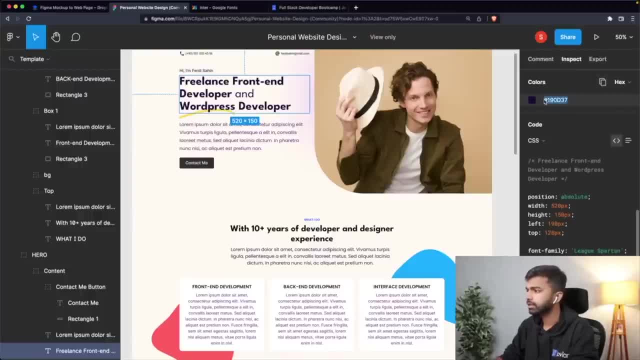 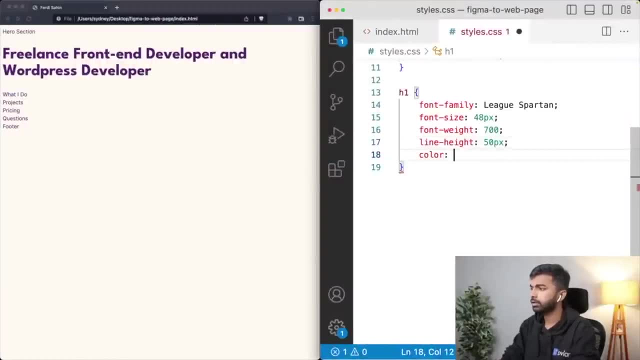 So let's just grab this color- one nine zero, D, three, seven- and let us grab this color and let us just go in here And let us set color to one nine zero, D, three, seven- And now we have the right color for the H1 as well. 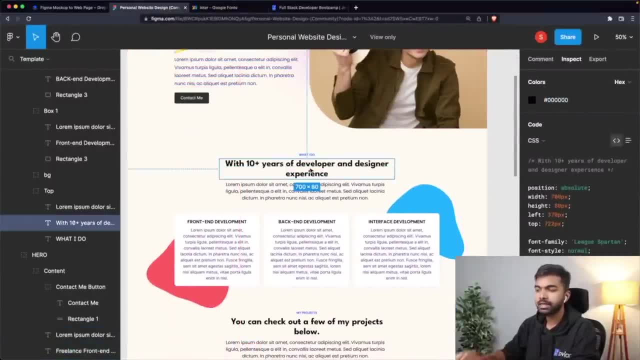 Okay, Great, Let's also fix the edge too. Let's fix this style as well. So I'm just adding in the basic styles that we added the body text background. We ordered the body font size. We added the body font family. 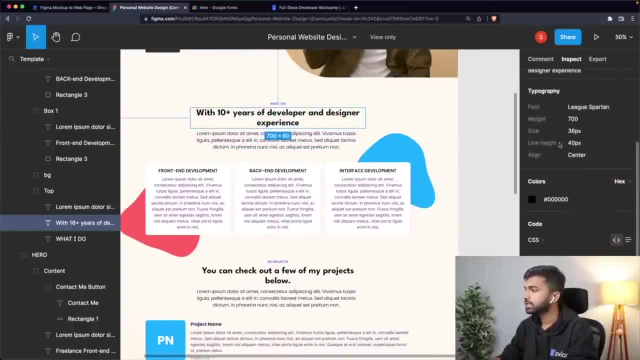 Let's add the font family for H2.. So with H2, seems like we are still using league Spartan. And how did I decide this is an H2? I'm just going by My gut feeling here. the biggest heading on the page should be an H1. 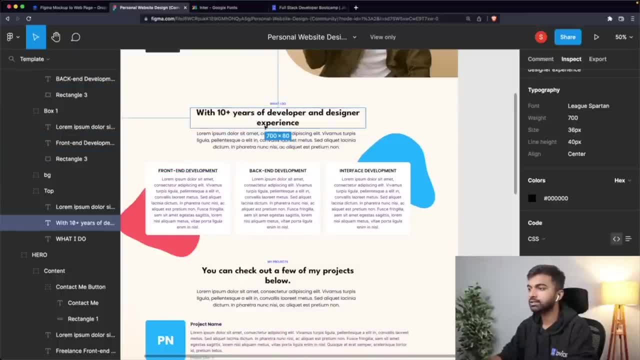 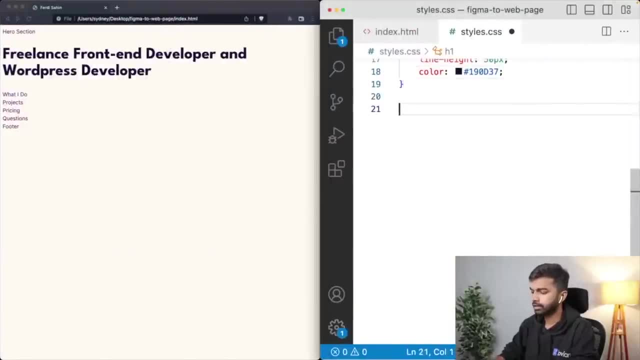 The second level heading should be H2, and then maybe these can be H3.. So we'll see. but for H2 here I'm just going to grab the typography settings and I'm going to create another H2 style And I'm going to again give it the right styles. 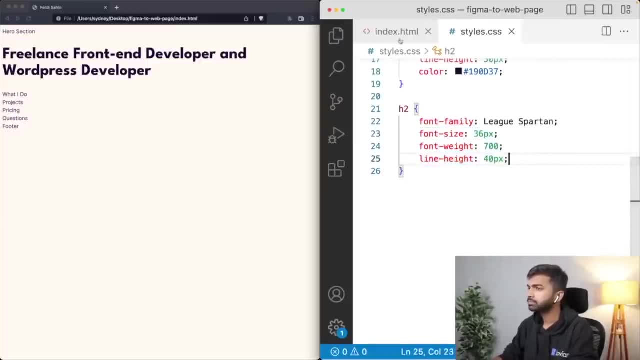 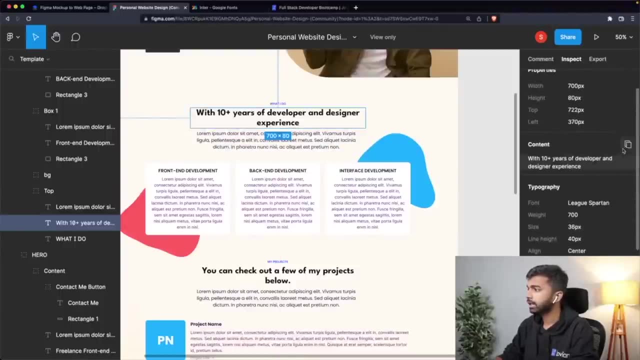 Let's get rid of letter spacing text line. We don't need that. And let's just verify that an H2 is loading fine as well. So with 10 years of experience, et cetera. So let me come in here and let me come in and let me just verify what I do, section. 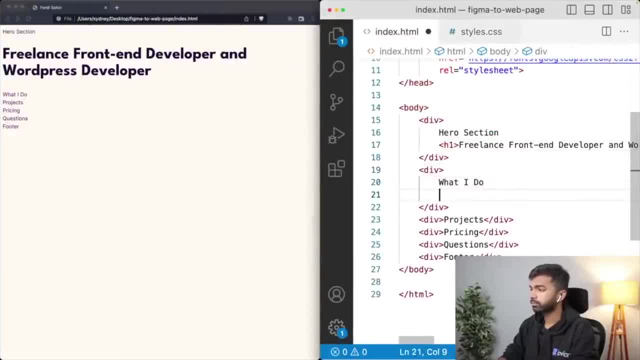 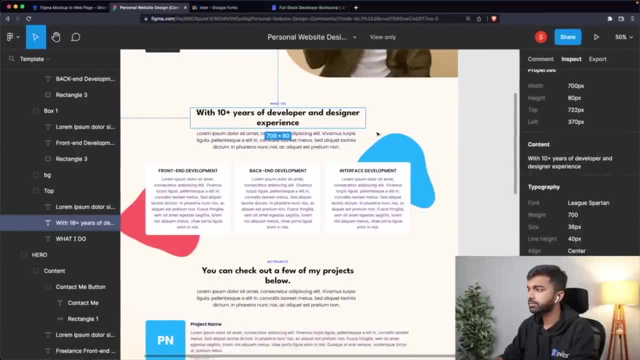 I'm just going to add an H2.. Okay, And let's reload. Okay, Again, the color seems to be off. Let's verify that we're getting the right color. So in this case, the color just seems to be black, or 0 0, 0.. 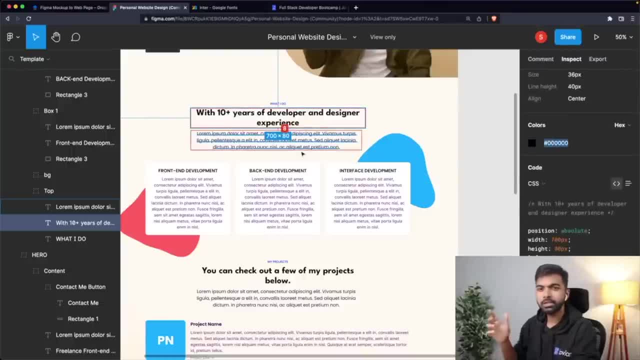 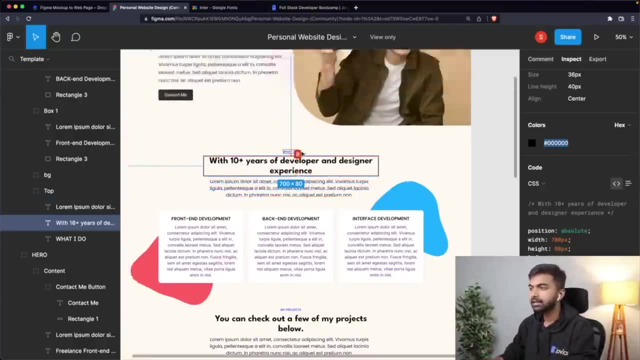 Yeah, So I'm just going to grab the color 0 0 0.. Ideally, although this could have been a mistake on the part of the designer, We do not mix Too many colors on a webpage, So my guess is that the designer may have intended to use the same color. one nine zero. 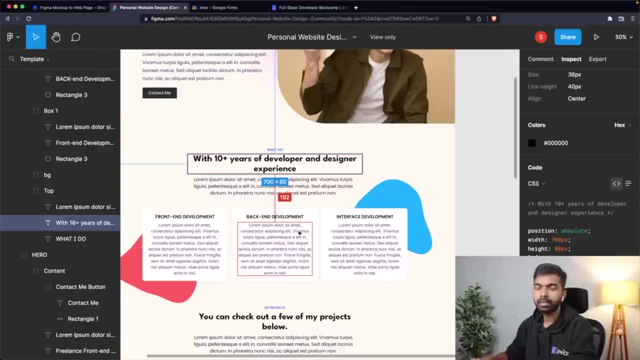 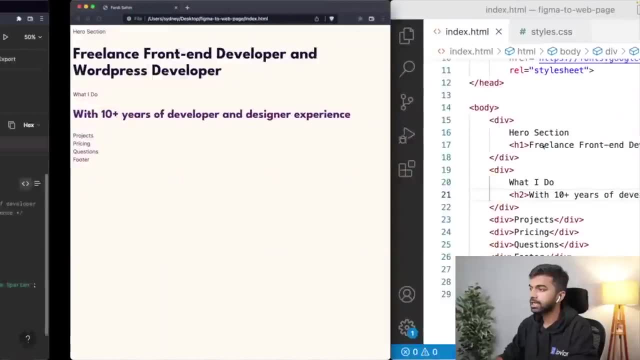 D, three, seven or, for these, H2 as well, but they probably just forgot to set it on Figma because these both look very dark. But in this case I'm just going to go with the design. whatever is on the design, Let's just replicate that. 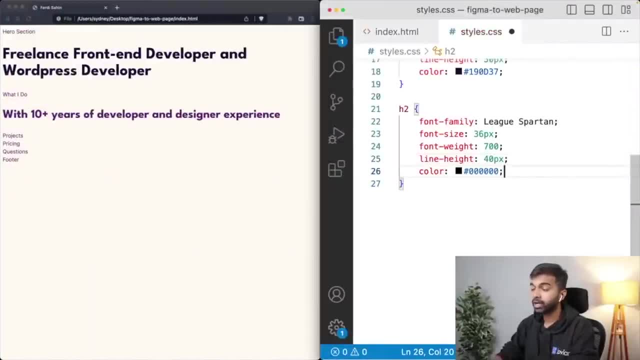 And that is a. that is a question that I might ask the designer- And, by the way, you can leave comments on Figma to ask questions- but or you can just check in with the designer directly. Okay, So now we have the H2. that is looking fine too. 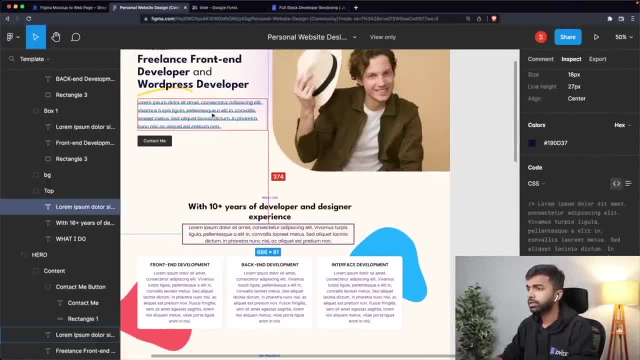 What else? Well, we have this body text over here. that is already inter. We have verified that, So let's maybe add this body text in as well. So, but the color, and the color also has been set for the body text. 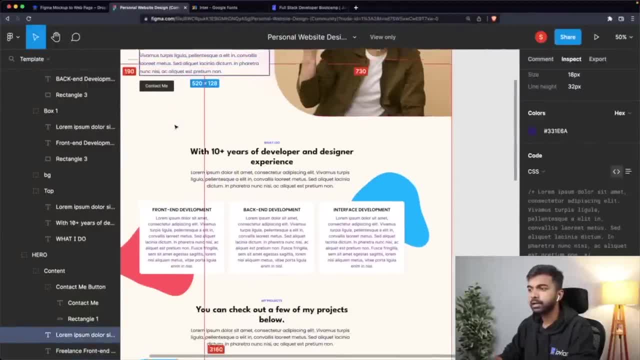 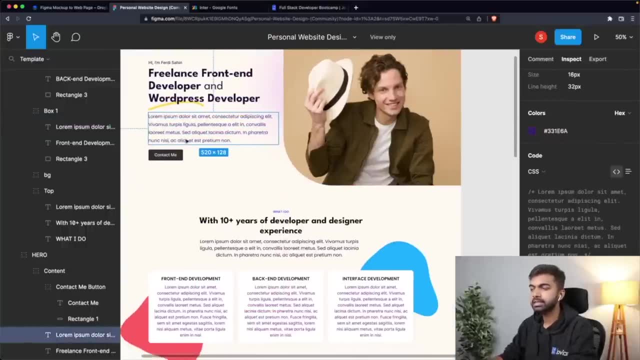 No, But this is not body text. exactly This is the body text and this we have made inter. This is like headline text of some kind. So this is big text. So what I'm going to do is I am going to set up a class for this and I'm going to take 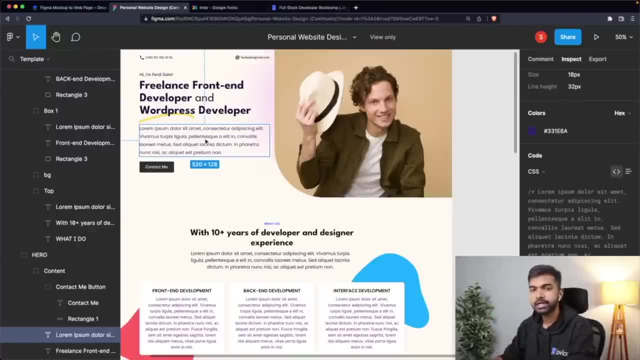 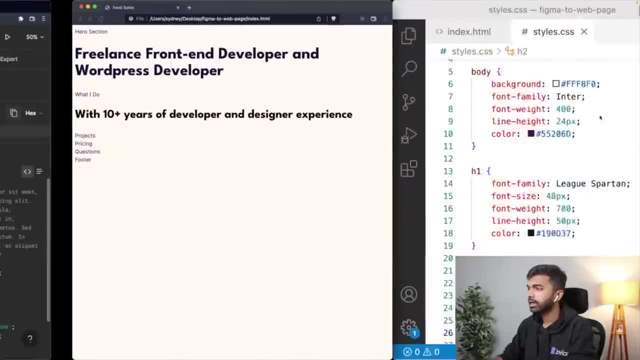 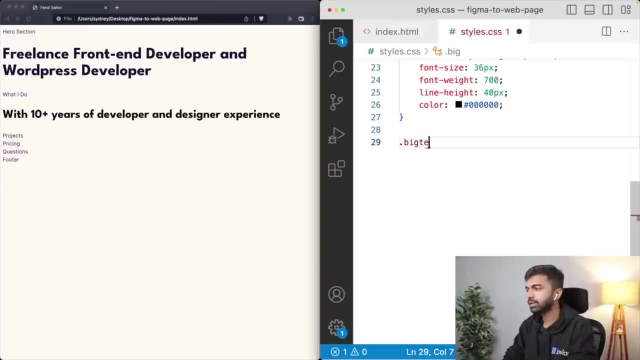 I'm going to apply those, those color and font settings to a class over here. Okay, So let me just grab this and let me grab this color and let me just call this class headline, So whenever I need to use, or let me just call it big text, maybe even headline may. 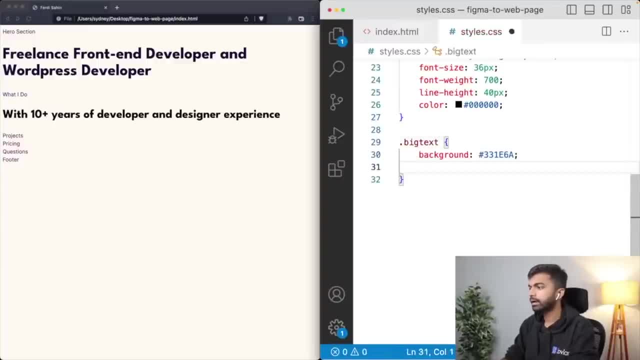 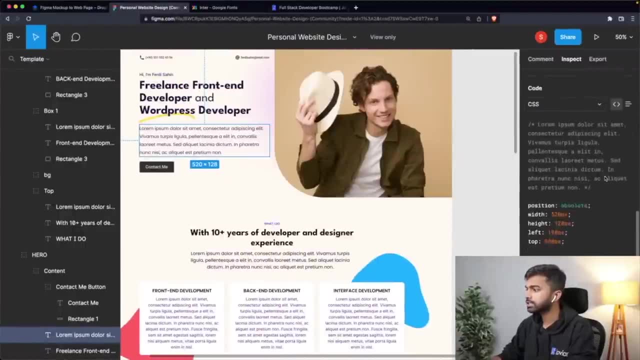 not be the right thing. So for big text, the background or the color that we want to use Is this: and what is the font size? Let's study the font size here. So the font is Poppins, The weight is 400.. 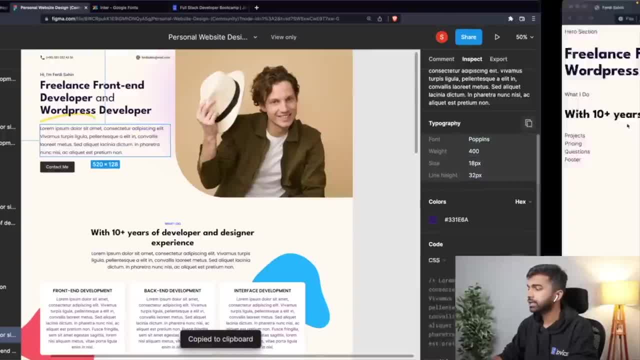 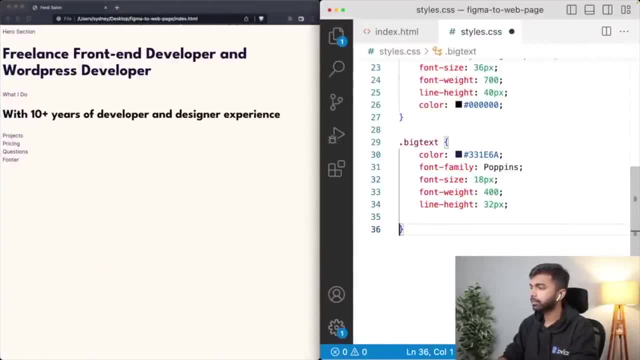 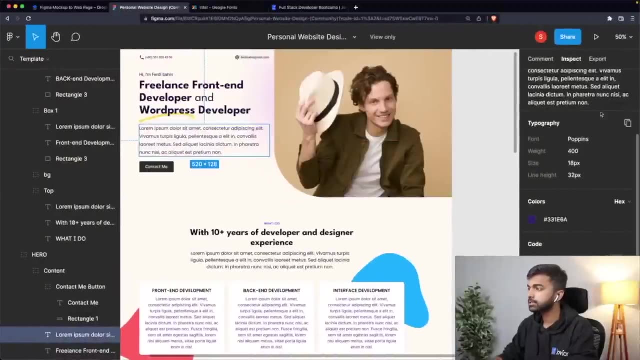 The size is 18 and the line height is 32 pixels. So let me grab that And let me put that in here as well. Yeah, And now we have the font size for big text. And if I want to verify if this big test, big text is going to show up properly, I can. 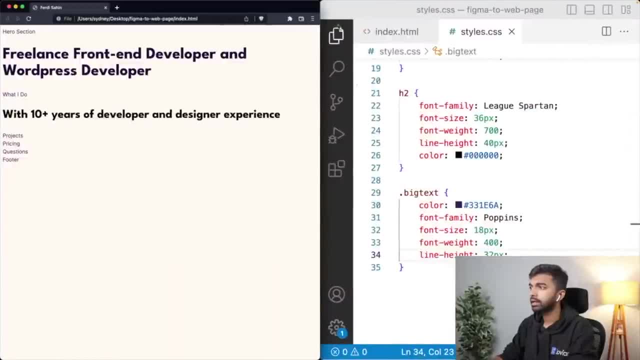 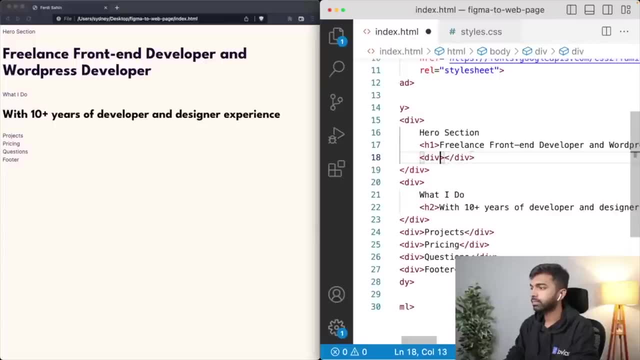 just copy this content, Okay, Over here, And I can come in into indexhtml under the H1.. Let me add a div and let me just give it the class big text and let me just paste the content here, Okay. 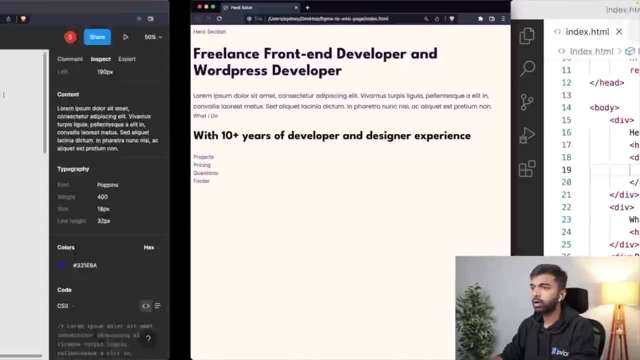 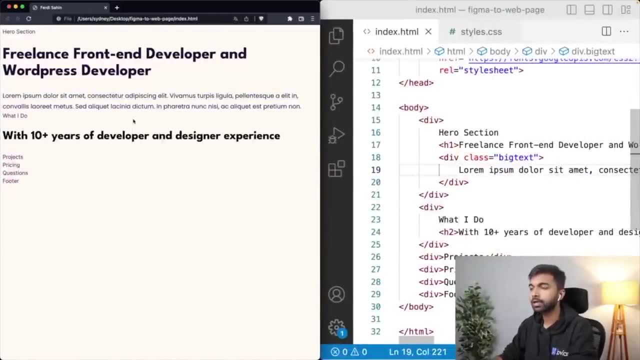 And I can verify that. Okay, This looks more or less like what we have here. lorem ipsum: yeah, it looks to be. it's definitely bigger than the normal body text. Okay, So I think we have set up most of the basic styles at this point. there are maybe there. 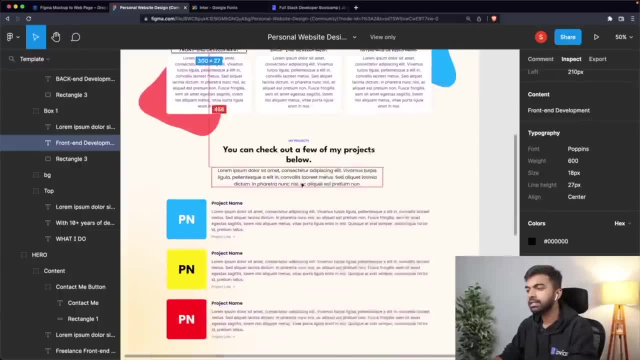 is this one style, and there is this one style here that we may need to deal with. Let's deal with them when we get to them, But at this point I feel I'm feeling pretty good in terms of the background of the page. 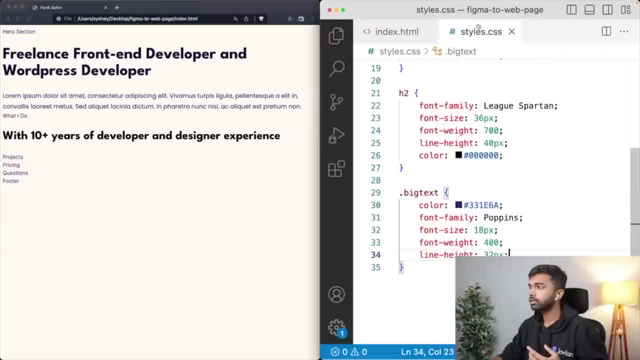 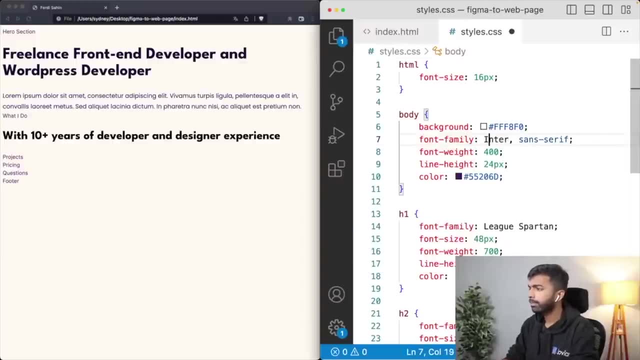 We've made a lot of progress. We've brought in all the fonts. We brought in the inter font, of course, which and we may want to give it like a, like a backup font in case the font is not picked up properly. 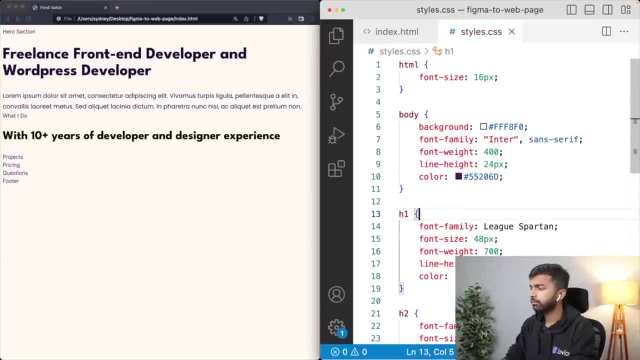 Then, similarly, we have the background Okay. So similarly we may want to give a backup font to leek Spartan as well. I'm just going to put sans serif here. So whenever you're putting in font families, it's always a good idea to also provide backup. 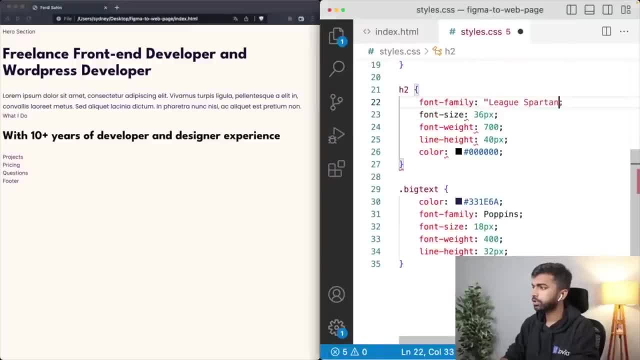 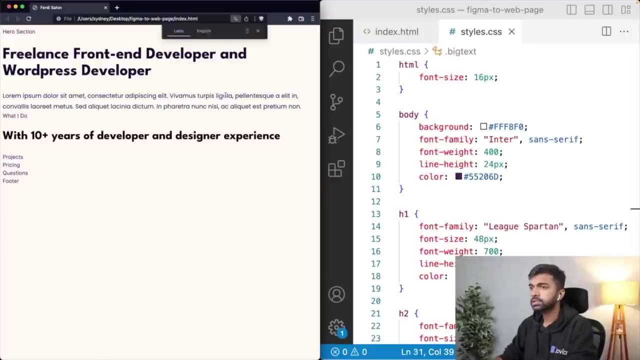 fonts, And let me also provide a backup font here, And let me provide a backup font here for Poppins as well. Okay, great, So that is going to make sure that our fonts load up properly. Okay, So we've provided the right backups. 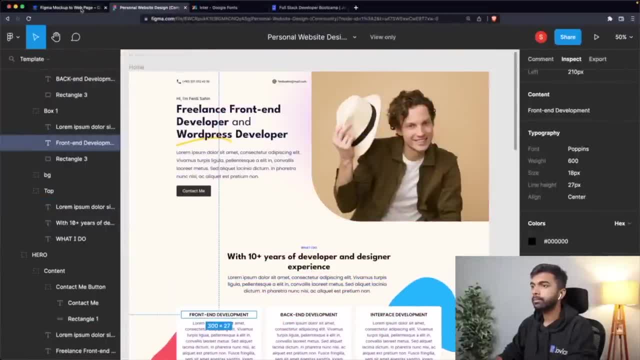 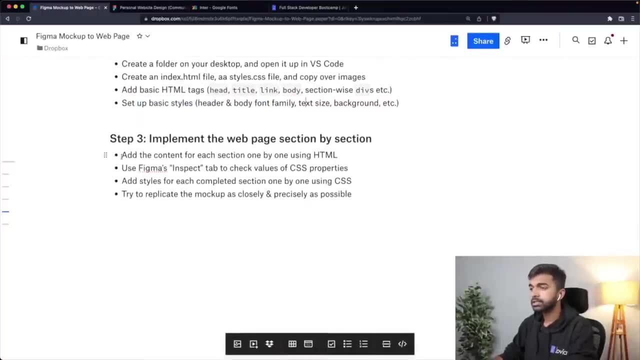 Fine, Next up, let us actually start building the web page section by section, because we've set up the basic styles- header, body font, family text size, background, etc. So let us add the content for each section one by one, first using HTML. 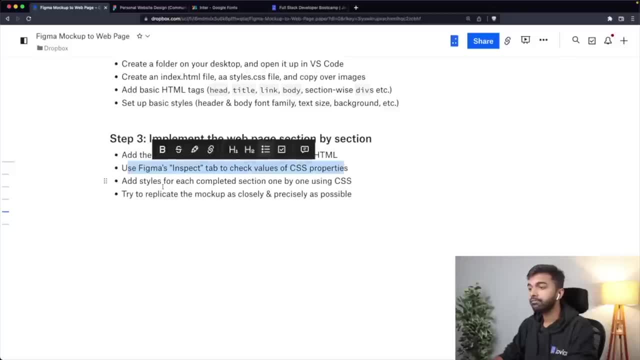 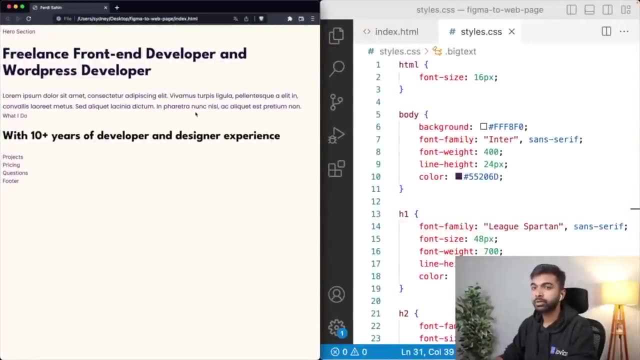 And then let us check the CSS properties for that content And then, finally, let us add styles for each completed section, one by one, using CSS. So we are going to go section by section. So I'm going to start with the hero section or the top section. 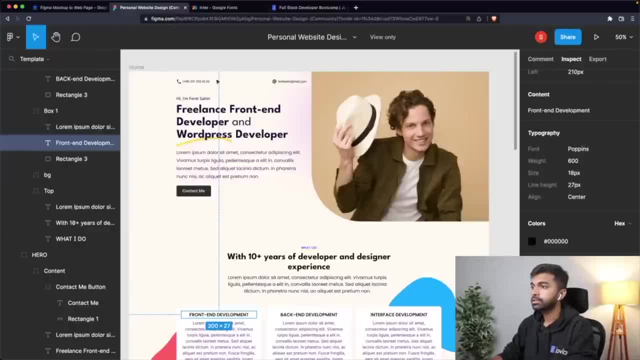 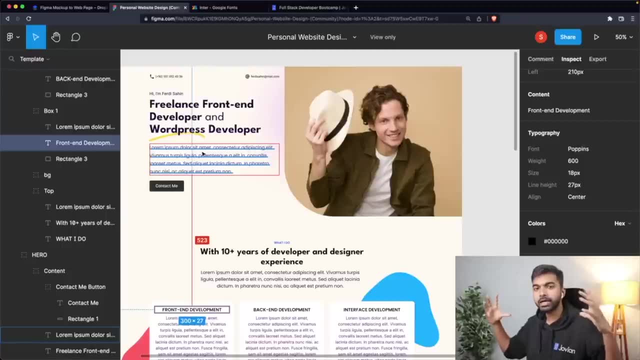 And I'm going to start by adding the content. Okay, So what do we have here? Well, there is this. the way you should approach these is: you should go in, you should go outside in. So this entire hero section here seems to be a box, right. 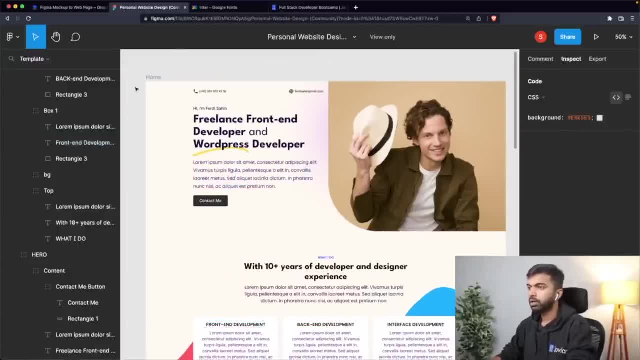 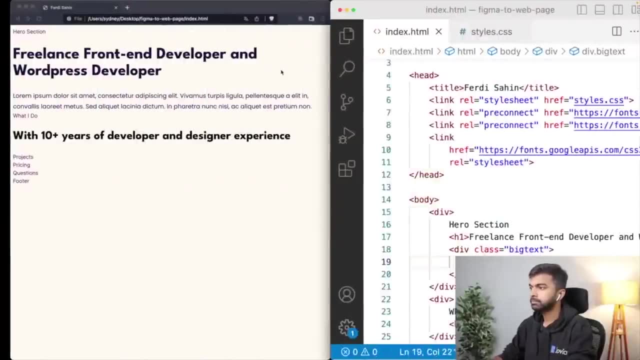 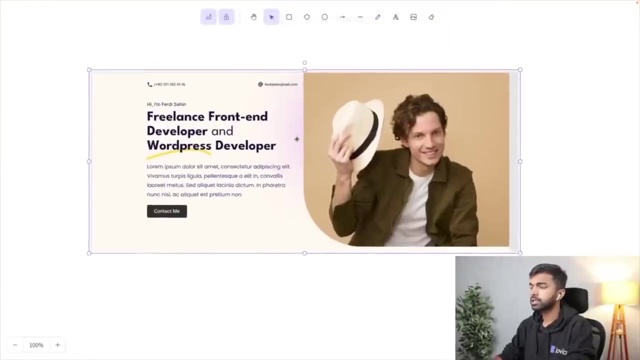 And then in this box, let me actually just copy this over to a whiteboard so that I can actually show you how I would think about something like this. Okay, so here is the design we have. Okay, So here's the design we have. 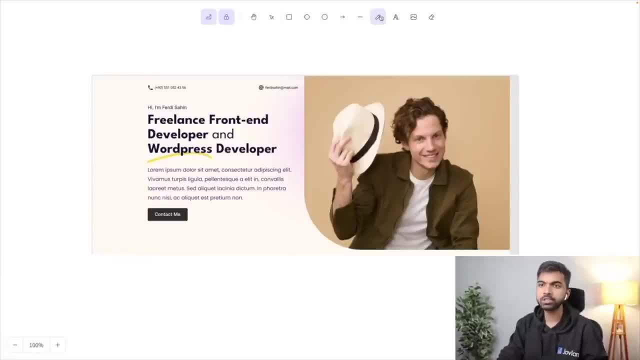 And now we're going to start annotating or start drawing boxes around this design. Now, in this design we have, first of all, of course, this entire thing is in a box, right? So this is our entire outer div, so to speak. 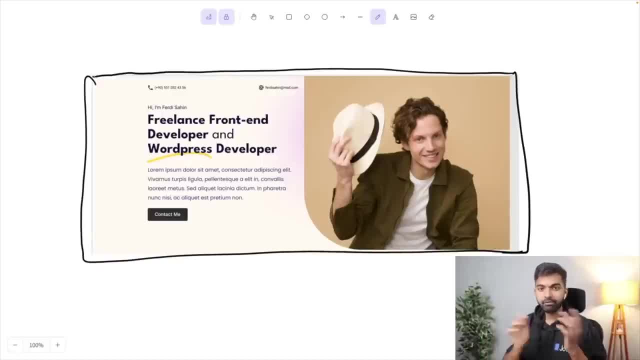 Now in this div there are two parts. there is a left half and there is a right half. So this is the left half. clearly, This is where a lot of the content lives. And then there is: this is the right half. 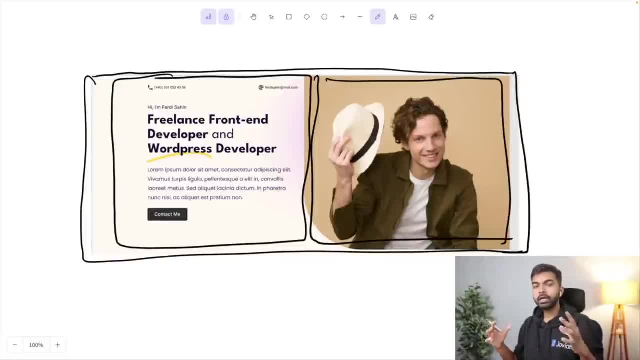 This is where we just have an image. Okay, So now you're already getting a sense that you need an outer div and inside that you need two divs: You need the left div and you need the right div. Now, in the left div, we can start again breaking things up. 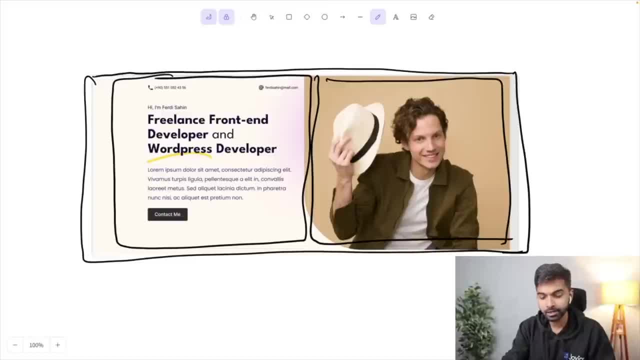 So what do you want to do? is you always want to see: okay, are things arranged horizontally or are things arranged vertically? So clearly, first in the outer box, things were arranged horizontally, So that will inform our CSS settings. Then, but in this left half, things are definitely arranged vertically. 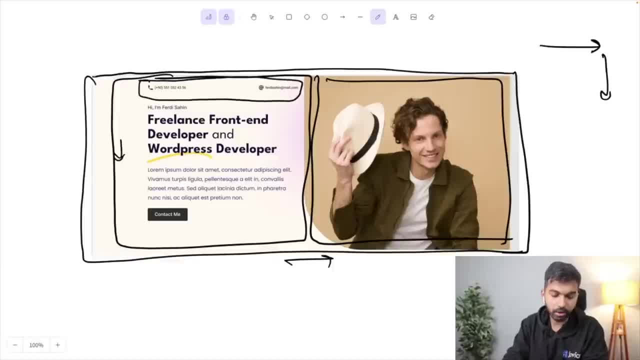 So there seems to be this one box that I can draw around this contact information, Then there is this one box that I can draw around this high section, And then there is this one box that I can draw around this section, which is just the. 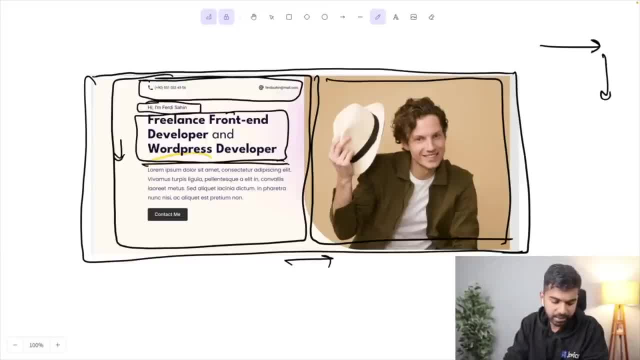 headline or the sort of the big text. And then there is this one box that I can draw around this big text, which is the body text, which is big in size, Okay, And finally there's one box I can draw around them. 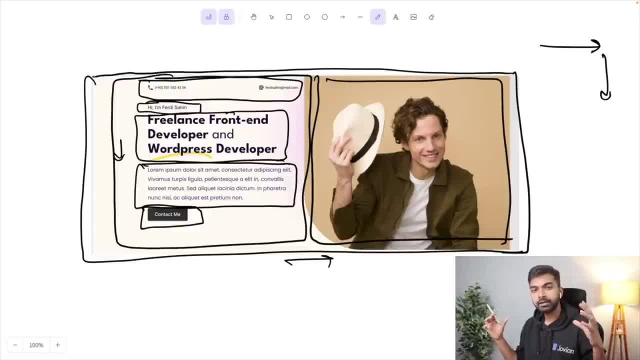 Contact me button. Okay, So at this point we actually have a very clear structure of the page and we can now start turning that into HTML content. All right, And I'm going to start giving some of these boxes IDs, just for easy identification. 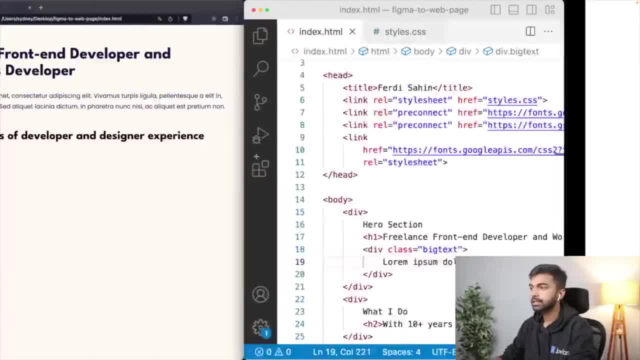 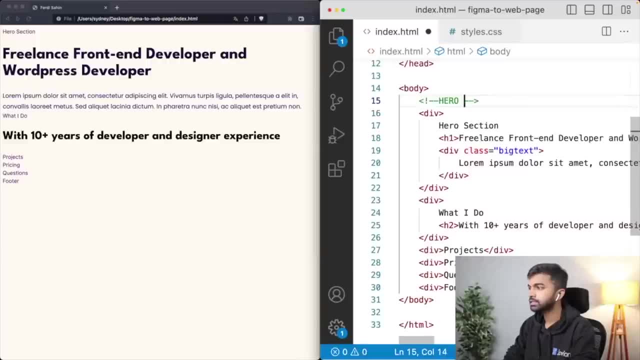 But another thing that you can also do is you can just use HTML comments. So let's do both, maybe, Okay? So first let's just create, let's just add an HTML comment here And let's say: this is the hero section. 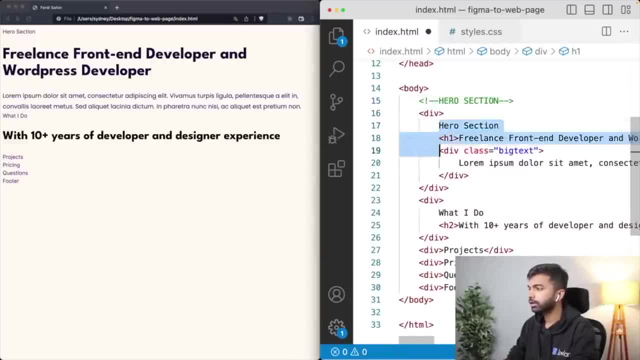 All right, Now in the hero section we have- I'm going to get rid of all of this for a second. I'm going to add it back later over time. in the hero section we have two boxes, So you always want to do the design outside in. 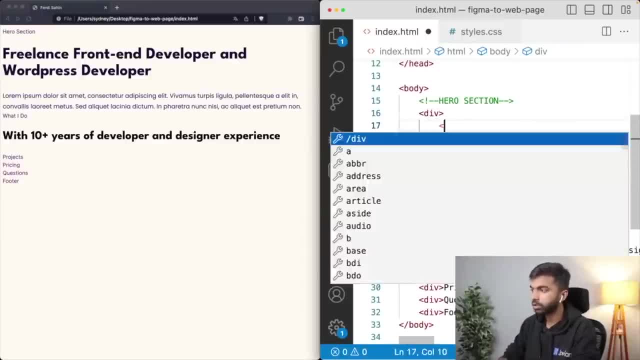 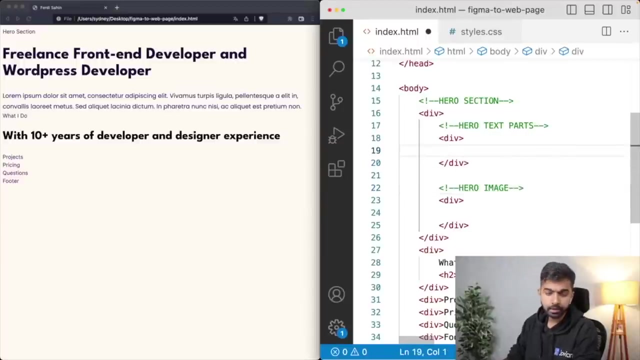 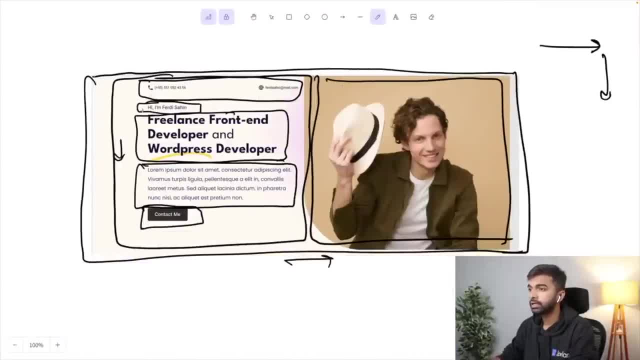 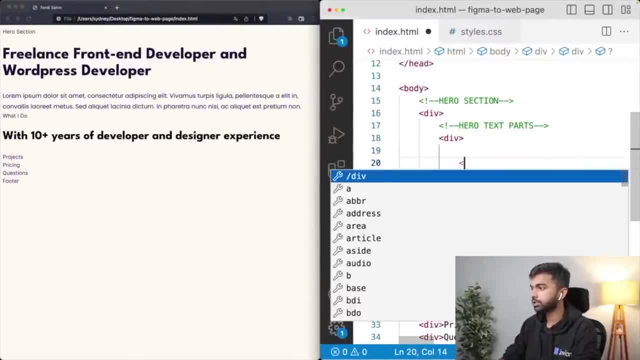 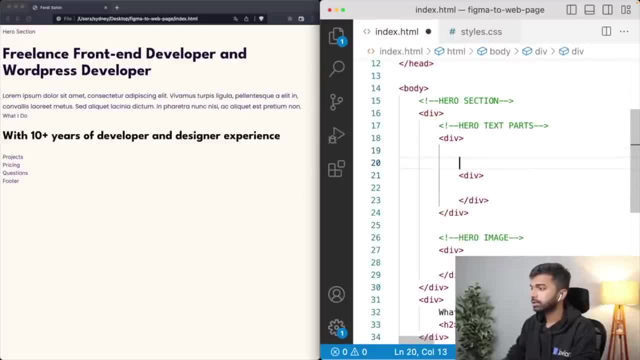 So one, two, three, four, five- Let me just add those in as well, just so that we have set up the structure before we are actually adding a lot of the content. So this is going to be. let's see. 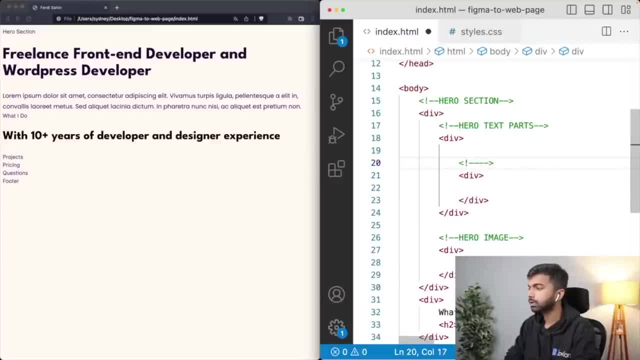 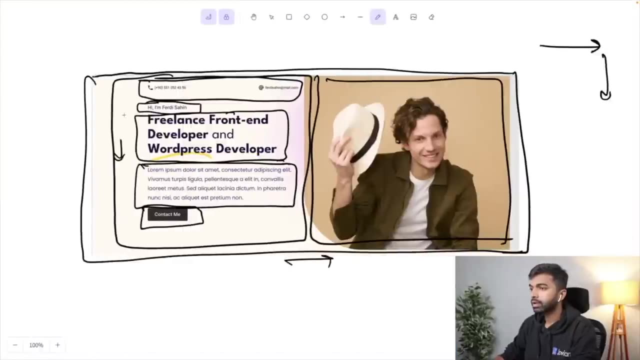 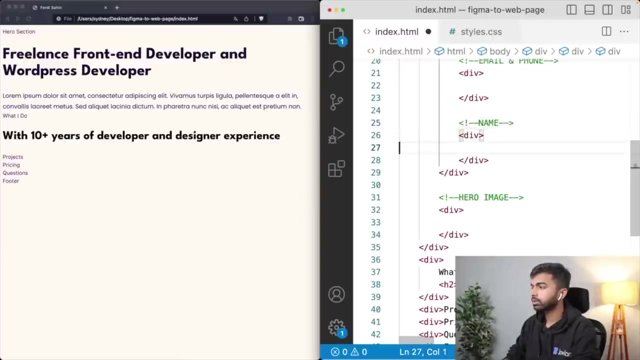 Okay, Okay, Okay, Okay. So this is going to be email and phone, And let's just put that in here, as we'll write that in here as well. Then, after email and phone, we have hi, we have the name, basically. 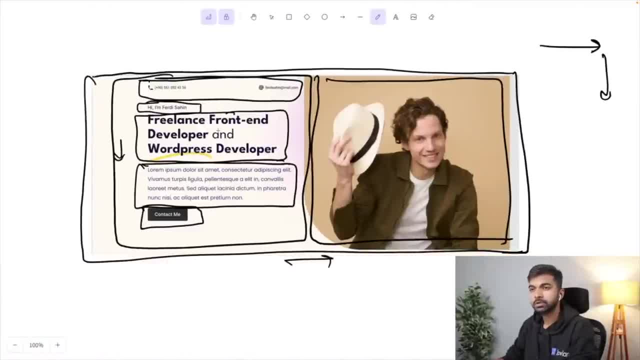 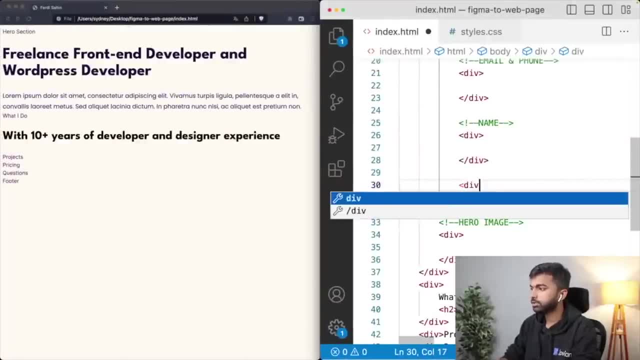 After the name we have this. Let me just call this like: Okay, H1.. So the H1 is going to be here. I'm going to create a div right now, but maybe later I might just replace that with an with. 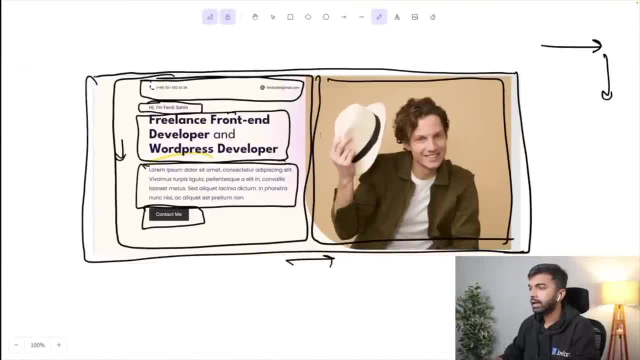 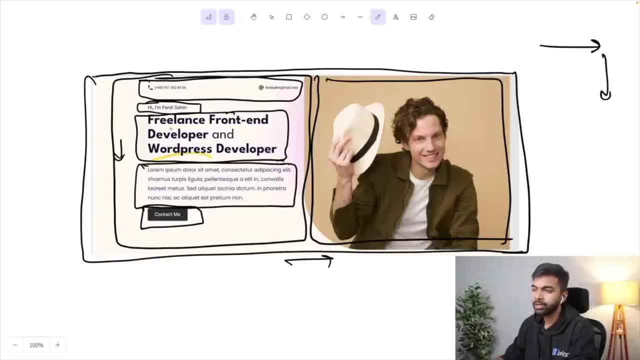 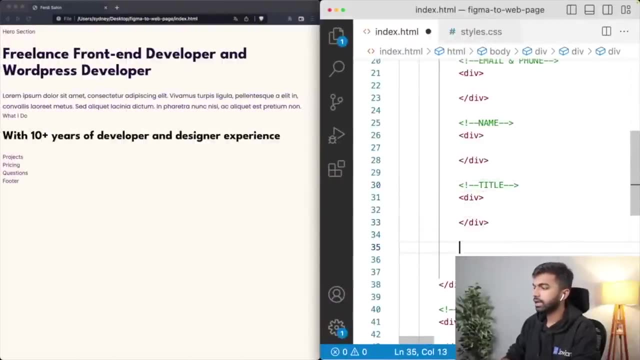 a direct H1 tag And then we have this explanation or this: let's let's call this subtitle, or let me call it title and subtitle, and then a button right. So let's call this title and let's call this subtitle. Okay. 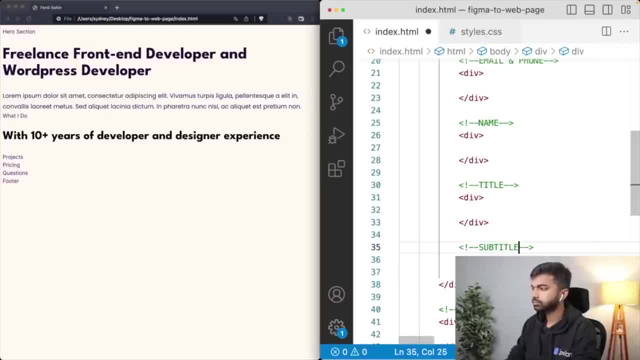 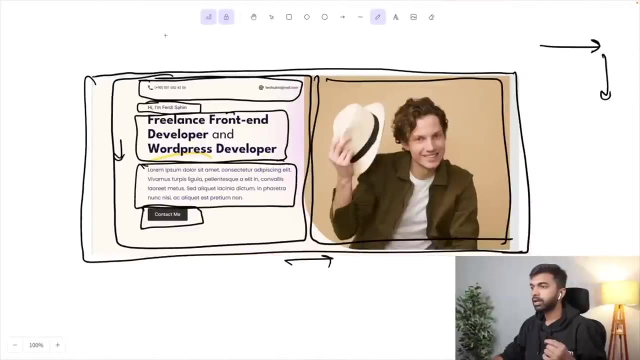 Okay, Okay. And then, finally, let's add a button. So there's a, there's going to be a button here, All right, So now we've set up the basic layout, We've set up a couple of, we've set up an outer div called hero, in which we have the 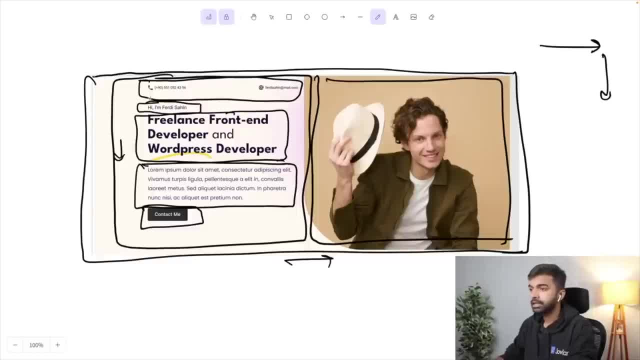 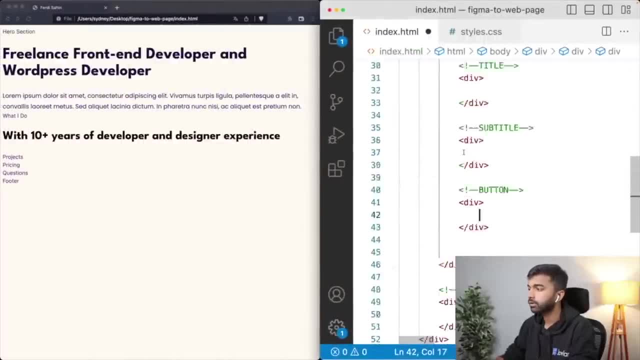 hero text, if we have the hero image div, and then in the hero text, if we have a bunch of divs- one, two, three, four, five divs for each of the sections within that section. Okay, So let's see. 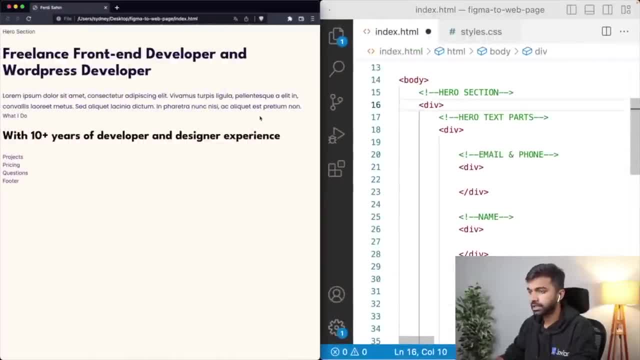 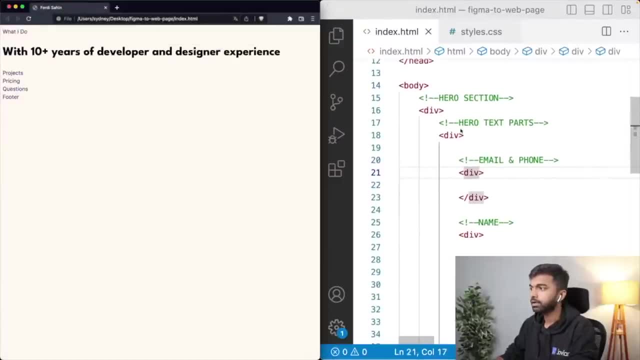 The first thing we need to do is, if I just reload the page, let me save this and reload the page. So right now we have nothing here. right Right now we have nothing in the heroes- hero section. So the first thing we need to do is maybe start putting in some content so that we can. 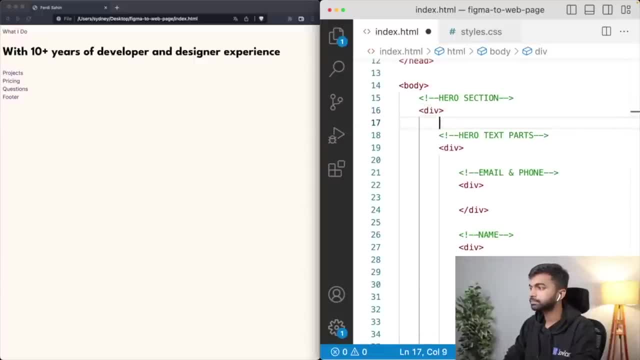 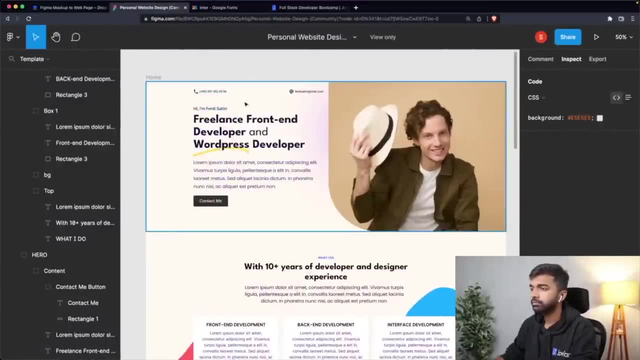 start getting a sense of where things are right. So this is the. maybe the first thing I'll do is I will put in the email and phone. So let me get the email And let me get the phone information. I will put in the email and phone. 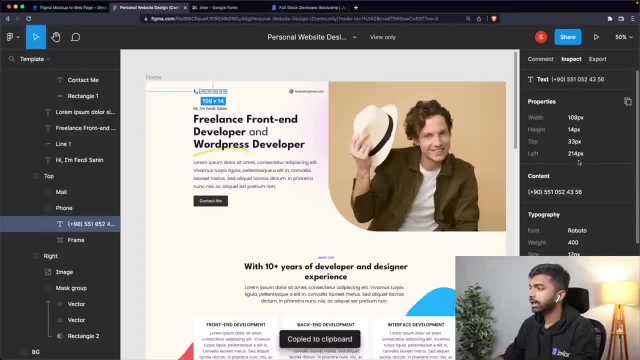 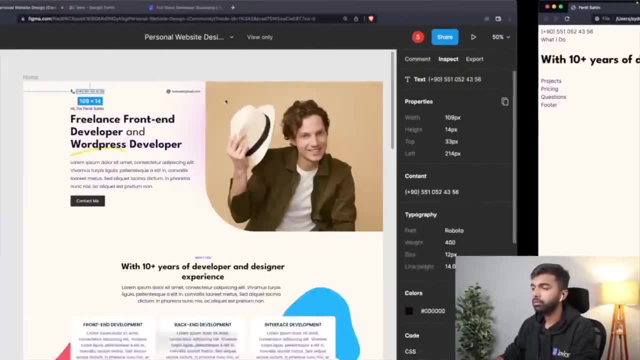 So I'm going to just go in here, I'm going to copy the phone information and let me put in the email and phone here. So let me just put put that in right now. Okay, So now we have the phone, then below the phone we have this text: hi, I'm Fardy Sahin. 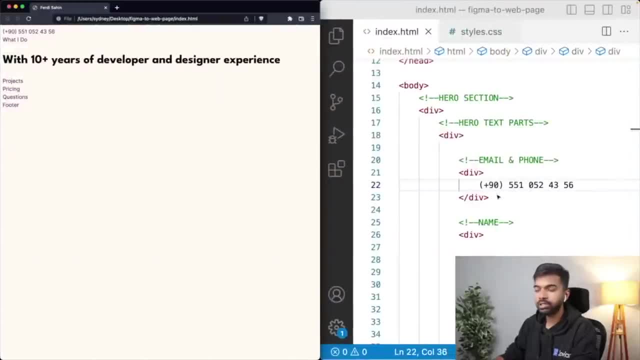 So let me just copy in the text of Fardy Sahin. I'll put the email shortly as well. Let me just I'll put in the email right now too. Let me just go in here. We'll figure out how to add the icon first. 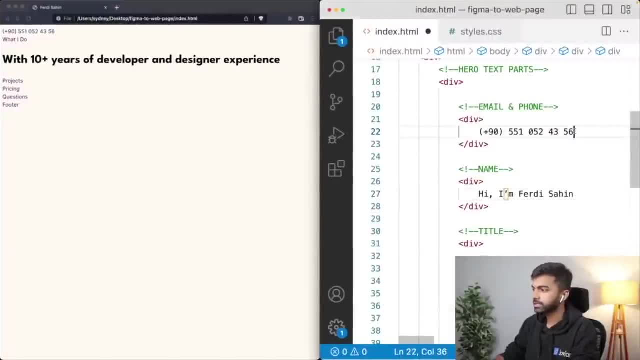 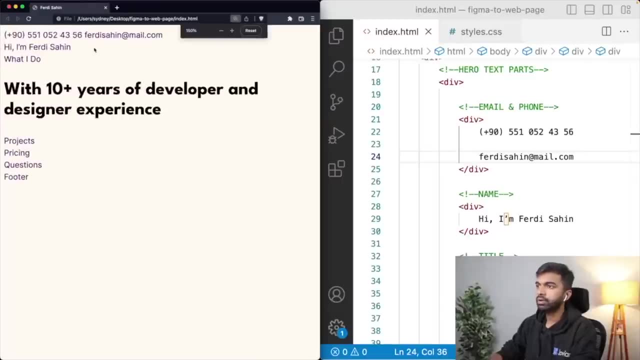 So the idea with any kind of web design is do the easy parts first and figure out the hard parts later. So okay, Now we've added the phone, We've added the email. I hope you can see here. I'll just zoom in for a second again. 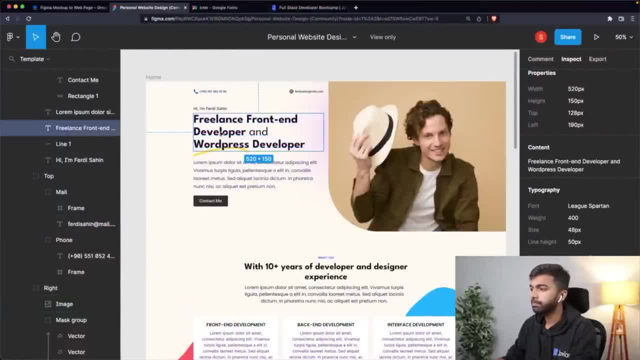 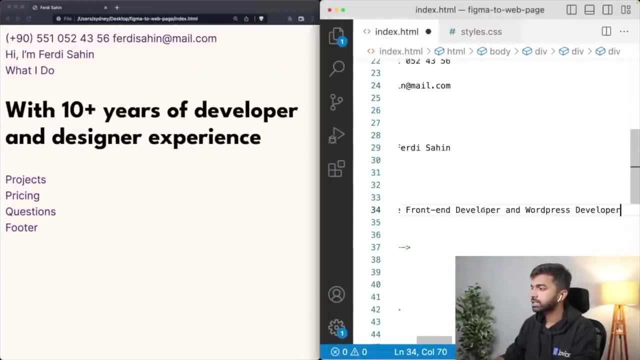 And then I've added that: Hi, I'm Fardy Sahin. I've added that part as well. Then let's add in this content as well, which is the freelance front-end web developer and WordPress developer. So this is an H1.. 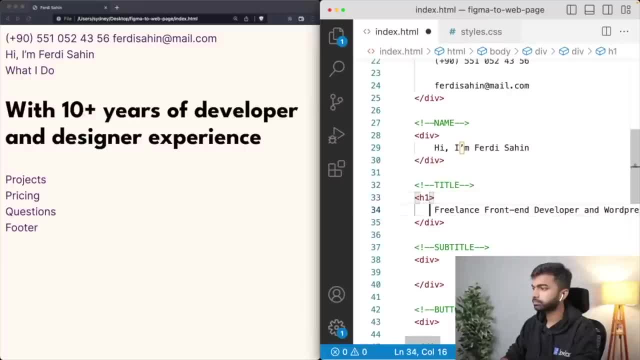 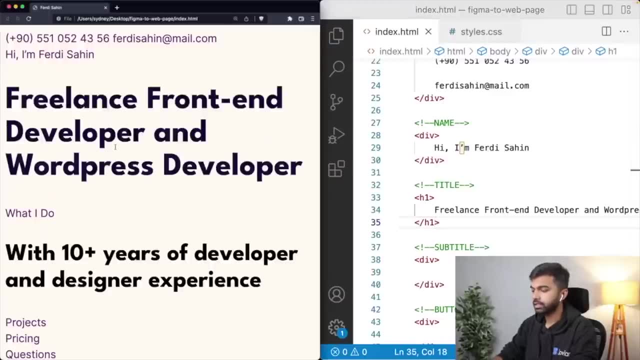 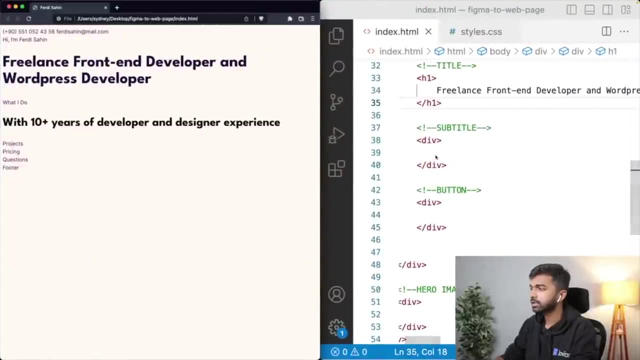 So I'm just going to add this in as an H1 directly. Okay, All right. So now we got the H1 here. Okay, In here as well, And then let us get this sub, this subtitle, So, which is going to be- I believe it is of the class big text. 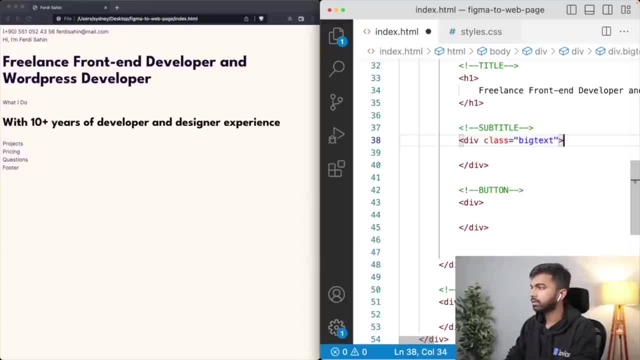 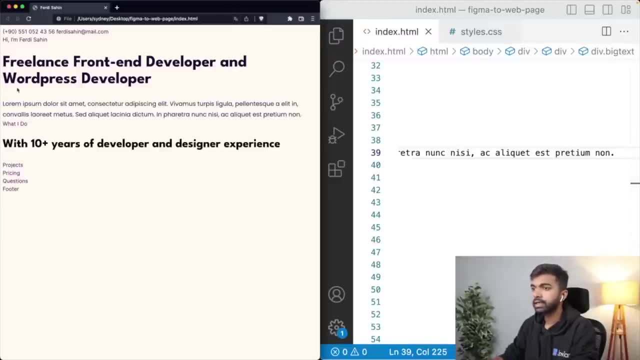 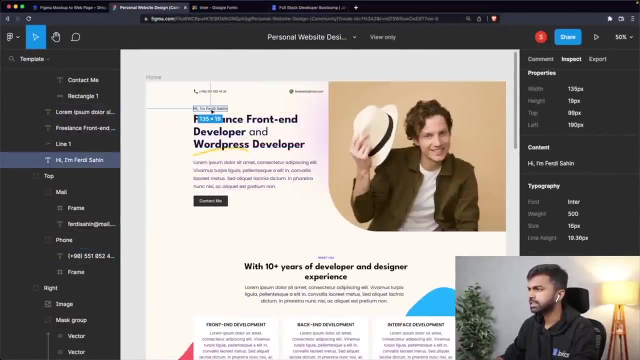 So let me just give it the class big text and paste the content. Okay, And now we have the class big text. So now, now we have the content starting to shape up. So we have the email and phone and we have hi, I'm Fardy Sahin, which is just body text. 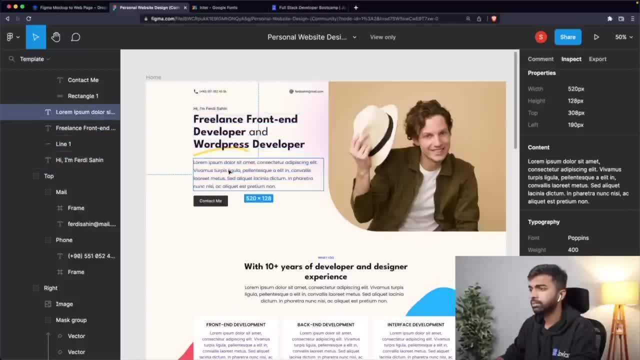 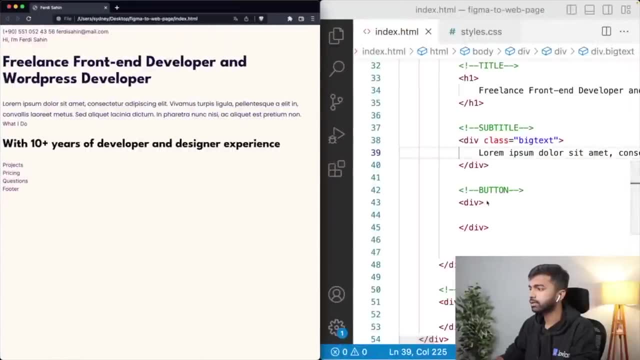 normal body text. Okay, We have a freelance front-end developer, We have this and we have this button here. So let's, let's add in this button here as well And this: so we have this button and this button button is called contact me. 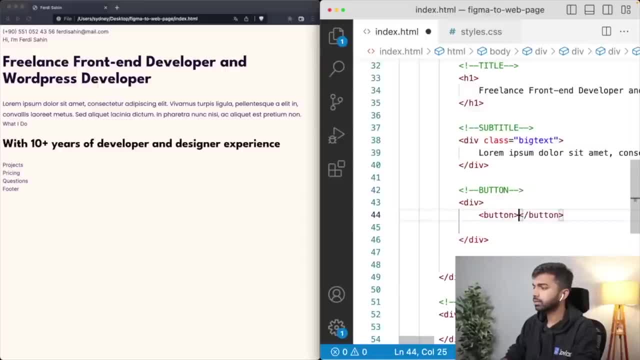 Let's put that in a div. Okay, So there's a contact me button, Perfect, All right. Now there is this image, this hero image over here. Let's come and get this. Let's grab this hero image as well. 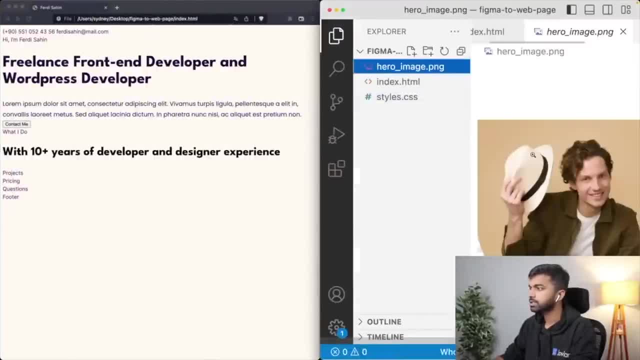 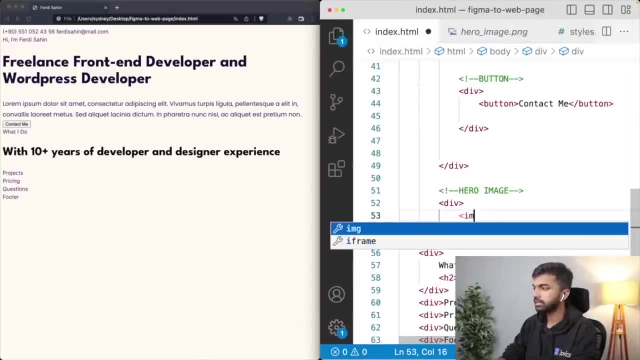 So we have already downloaded this image. If I show you here, we have this hero image that has been downloaded already, So I can go in and I can just import or use this image using the IMG tag. So IMG SRC equals um hero image or PNG. 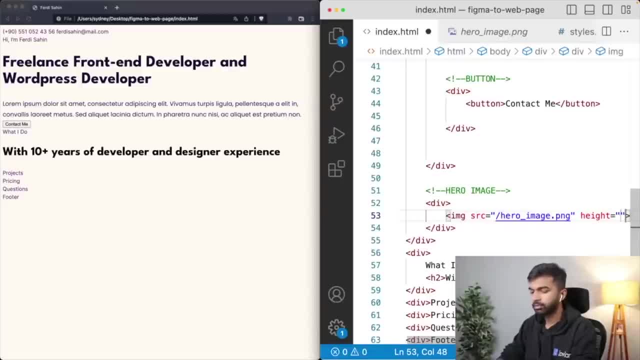 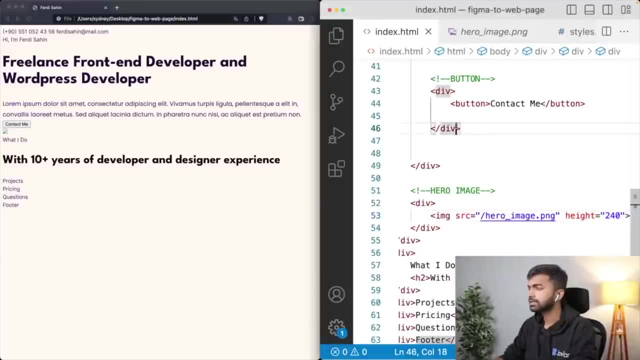 And let me just for now, let me just give it a height so that it's not too big, but we'll adjust the size later. So let me give it a height of two, 40, and we'll adjust specific exercise sites later. 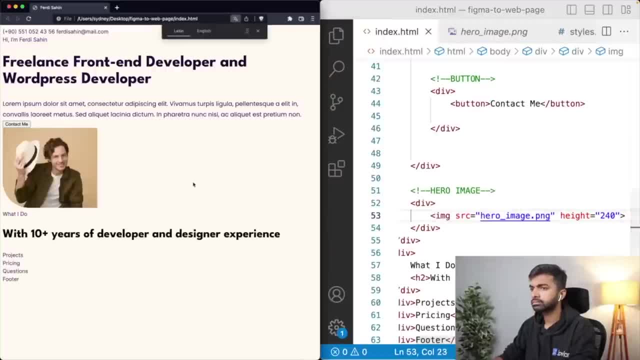 So hero hyphen image dot PNG. Okay, Yeah, There it is. So now we have the image here as well. Okay, Perfect. So now we are getting to a point where, for the first section, we have all the content. Now the next step is to maybe start aligning things a little bit. 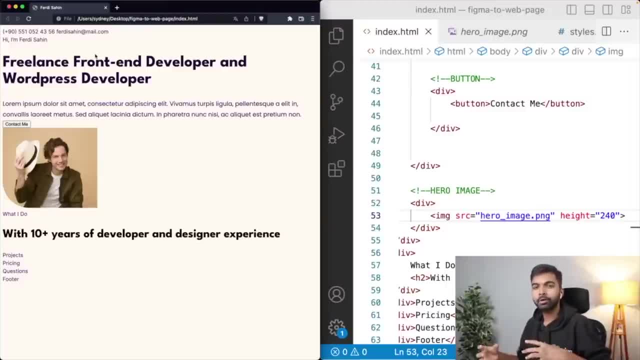 Right, And of course you can go back and forth with this. You can add a little bit of content, do a little bit of alignment, and add a little bit of content, do a little bit of an alignment. But just to keep things simple, for now I'm adding the entire section content and then 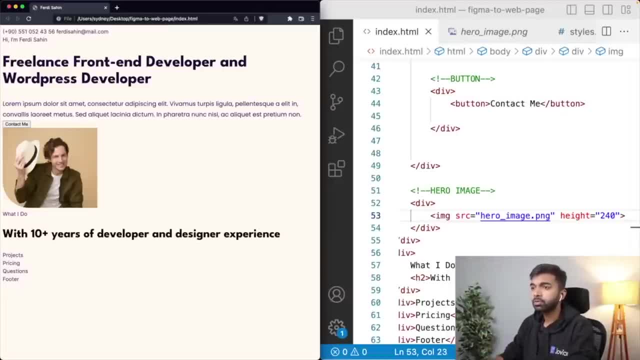 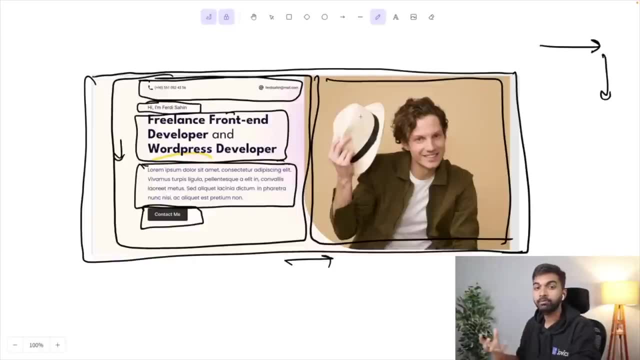 I'm going to style it Um, okay. So we, first of the first thing we want to do. What we want to do is we want to show these two diffs horizontally and we want to maybe make them both take up 50% of the screen area. right, 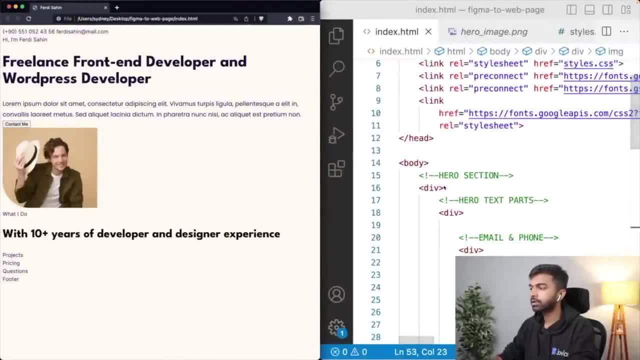 So to make things horizontal- and you can always look this up, You can always say how to show two divs horizontally- but let me just give this a class, or let me give this div an ID called hero section and into the hero section. 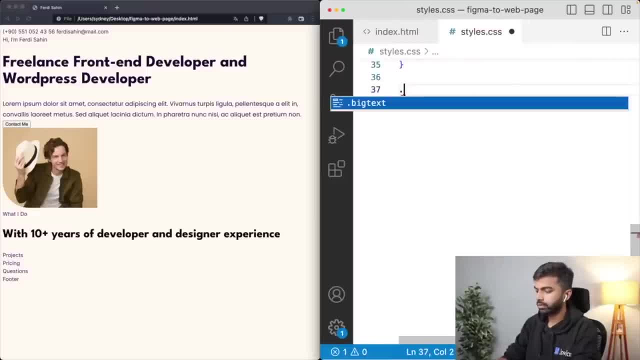 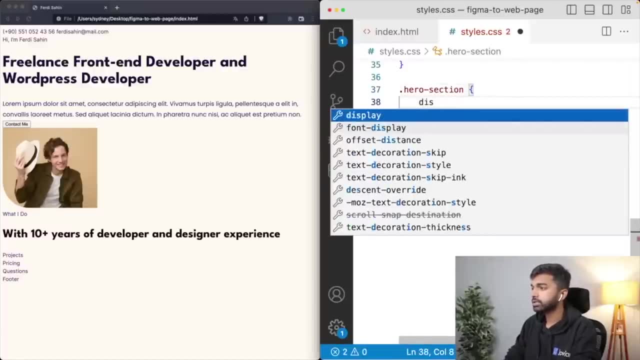 I'm going. I'm going to go into styles, dot, CSS. Okay, Okay. So in the hero section I am going to say display flex. So this is a quick trick that I want to tell you Anytime you want to show the children of a div horizontally. just said display flex. 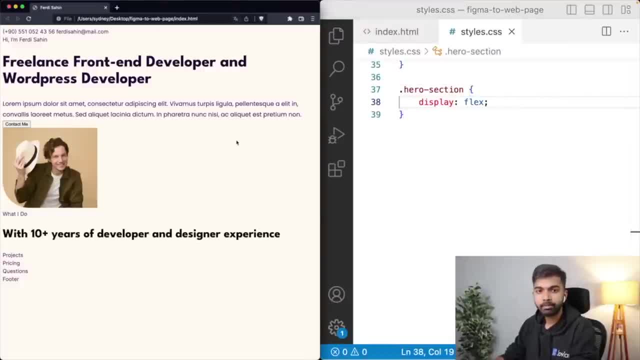 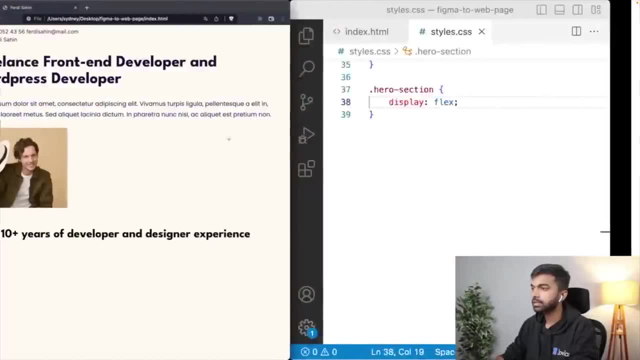 Okay, And just as I do that, nothing seems to happen. because inside it we have these two devs and we want both of those inner devs to be taking up 50% of the space, Right? So let me just give them some IDs as well. 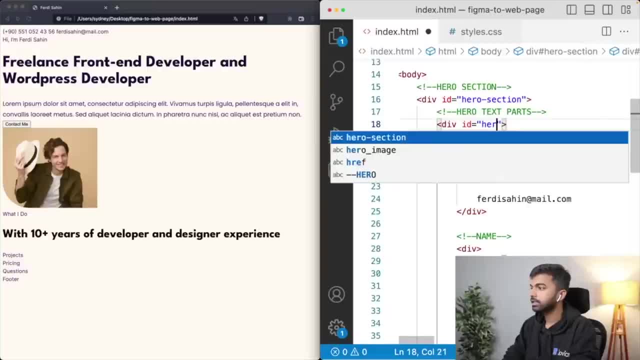 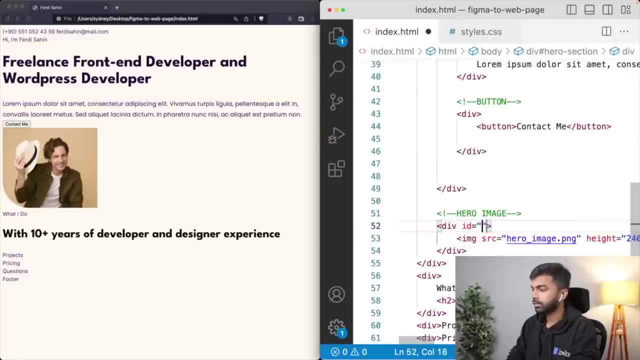 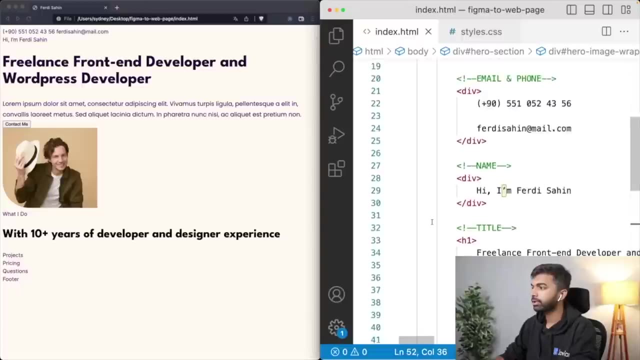 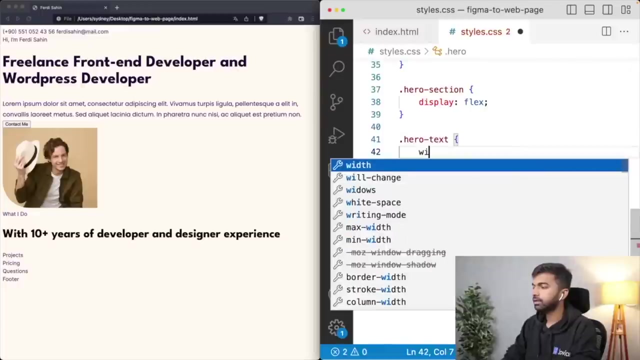 So let me say: let me give this an ID: So hero text. and let me give this an ID hero image wrapper, because it's not exactly the image tag itself. This is a wrapper around the image, So hero text. let's give that a width of 50%. 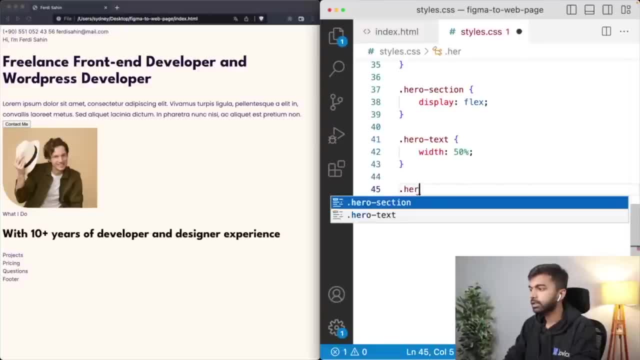 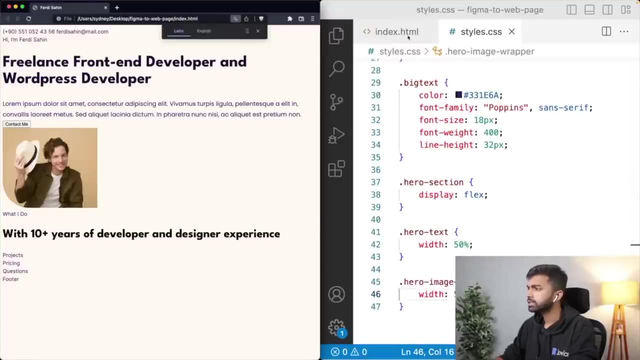 So it takes up 50% of the parent's weight, And then we have the hero image wrapper. Let's give that a width of 50% as well. Okay, And let's see what happens. Okay, Nothing seems to have happened, which is strange. 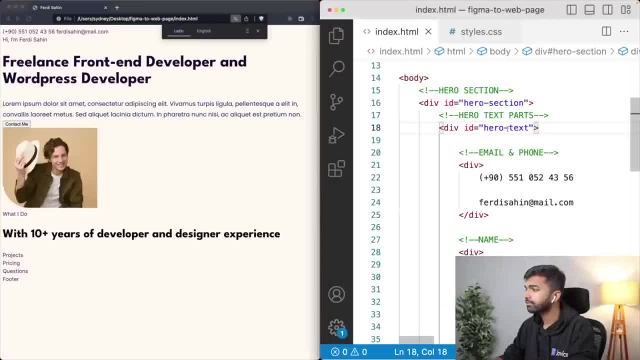 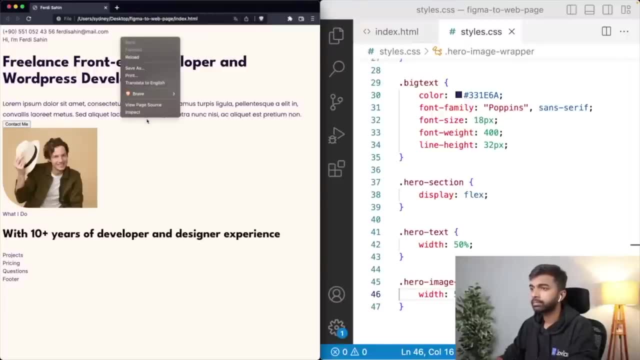 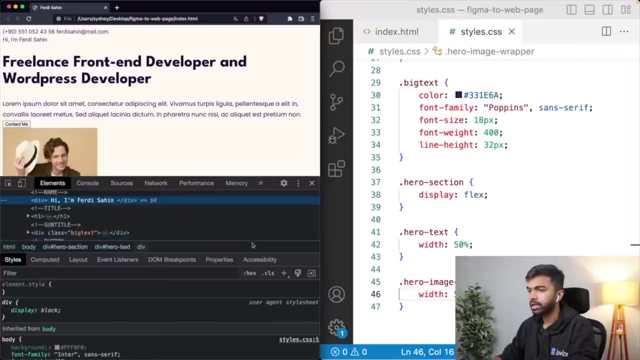 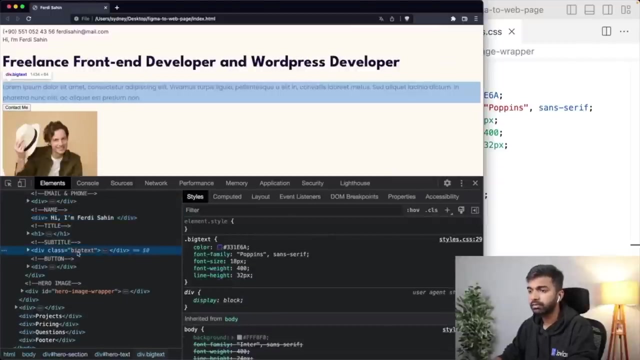 So these are the issues you run into when you are doing things live. At this point, the way I'll debug this is: I will just right click here, I will check, inspect And- let's zoom this out a little bit- And I am going to then- yeah, I'm going to then maybe just check whether the div actually 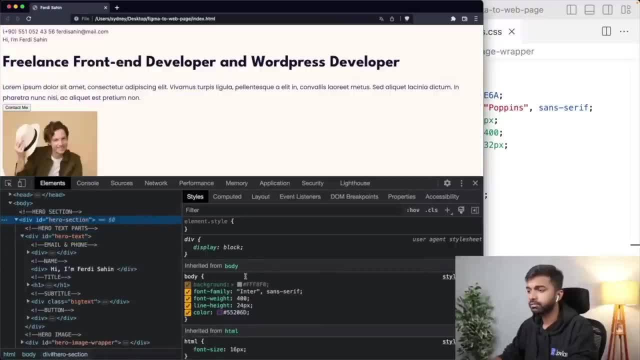 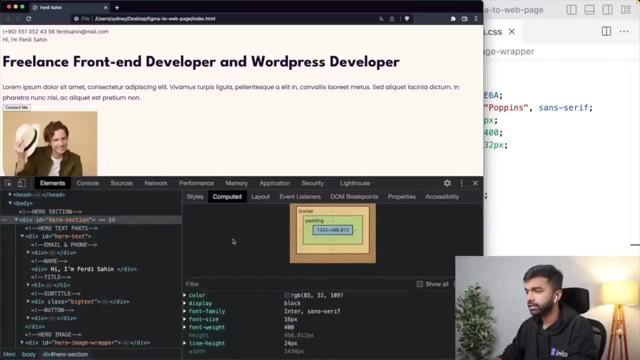 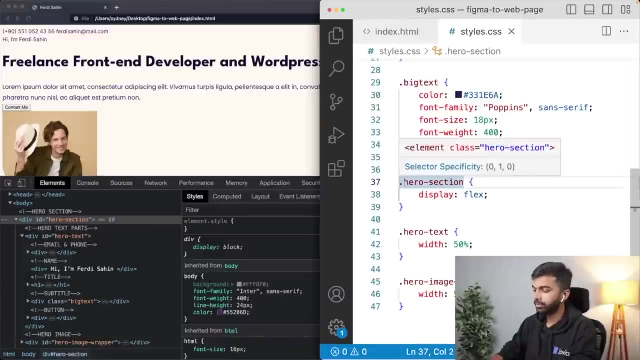 was added properly or not. So we have the hero section, div, and the styles don't seem to have been applied. Why was the style not applied? Hero section? Oh yeah, So the styles are not applied. Okay, So I have to select by ID. 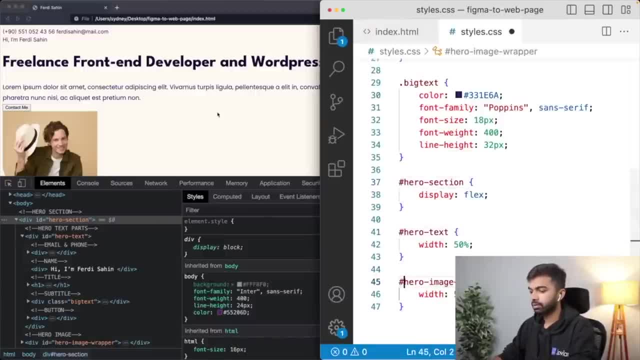 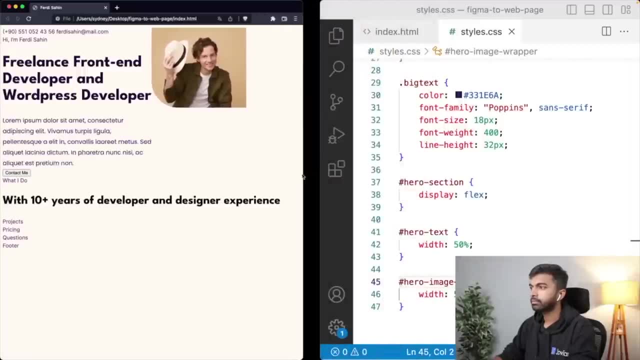 So let me just make that hash instead of dot, Okay, And let's reload the page. And now you can see already that both of these seem to be taking up. So this is the hero text section And this is the hero image section. 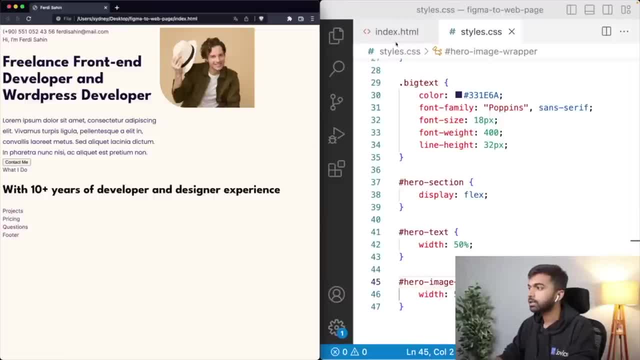 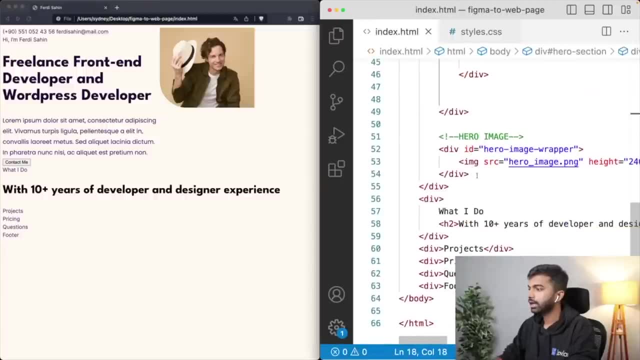 Both of these seem to be taking up about 50% of the space. Now, of course, this image itself is not taking up the entire space, So I might want to come into the image here And maybe let's just put the image. let's get rid of this div. 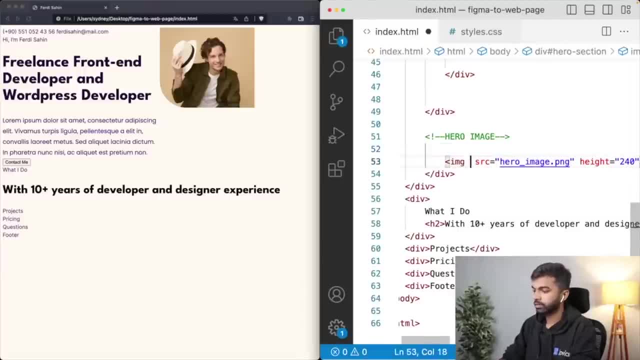 And let's just put the, let's just give the image an ID And let's just call it hero image. And this is one question that you will ask yourself a lot: When should I be using a div? When should I not be using a div? 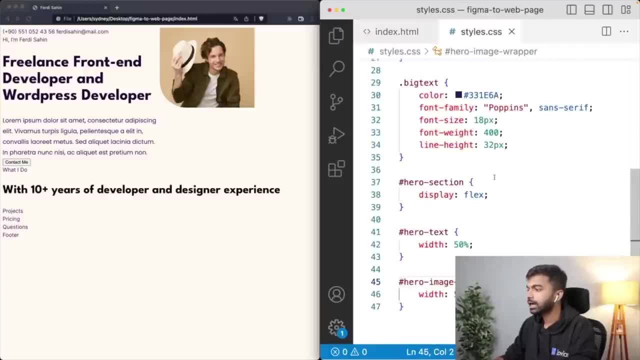 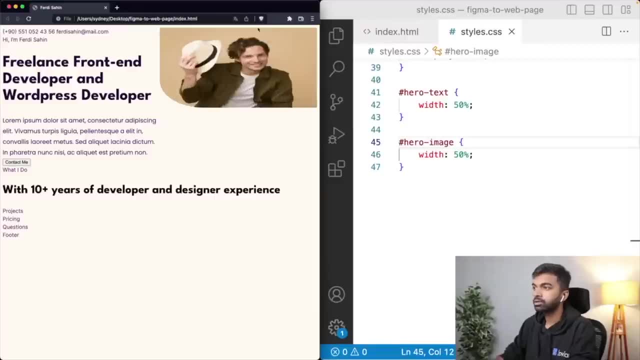 The answer is: whatever does the job, but you can start, start with something and then modify it as you need. So let's just give the hero image a width of 50%. Okay, so now the hero image has a width of 50%. 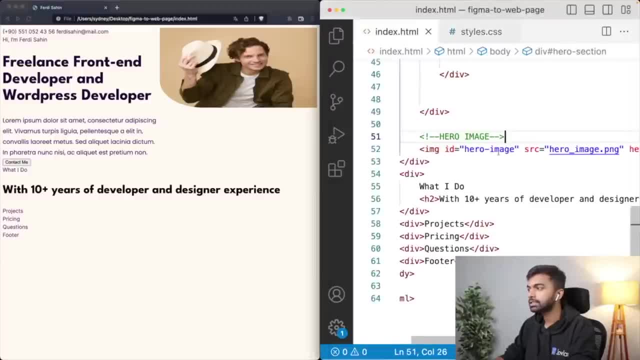 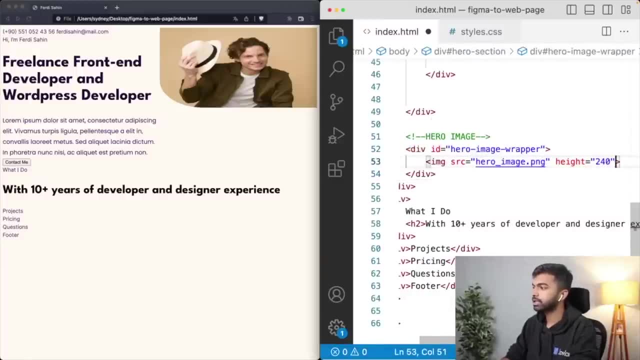 That's fine, But that is not fully doing the job for us. So I think I'll just revert to the old style And then I'll just apply some styles to the outer hero image. So let me go in here, let me remove the Oh, that's because I had the height. 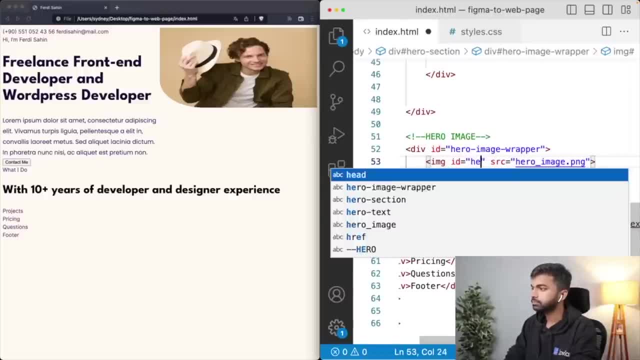 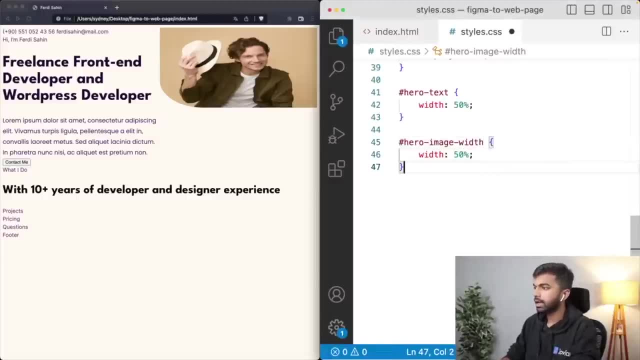 So let me add the ID hero image here. So I keep my hero image wrapper at a width 50%, And now I'll go into my hero image And I will give it 100%. So it's going to take up 100% of the parents width. 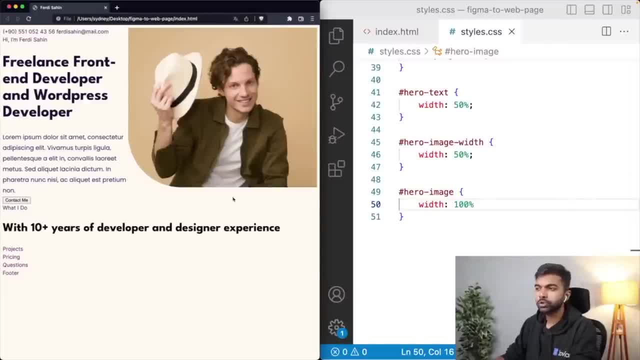 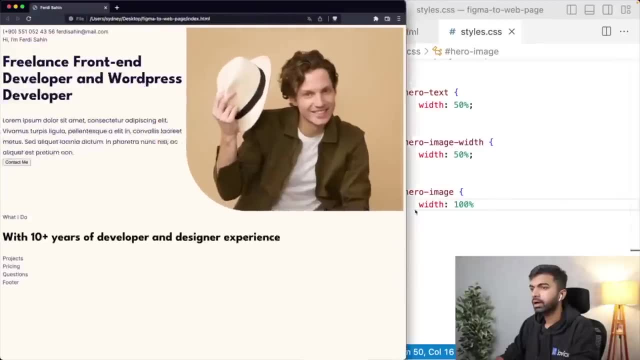 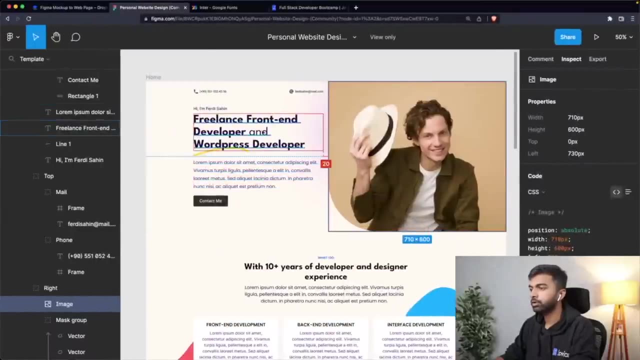 Okay, So now the hero image should be taking up about 100% of the parents width, which it seems to be doing. However, you can see that this parent itself, this entire thing, is kind of spreading across the page, which we may not want. we may want to just put a maximum width to this entire. 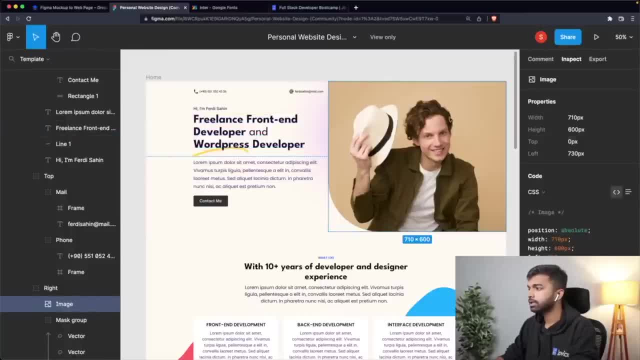 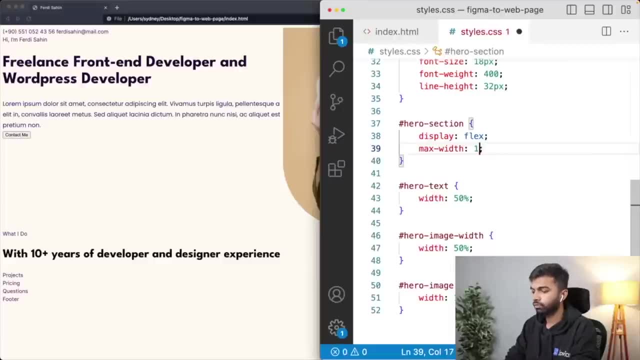 to this entire section And I think the maximum width that we're putting here- Okay, The maximum width that we're putting here- is about 1440 pixels. So let me just set the entire maximum width for the hero section to 1440px. 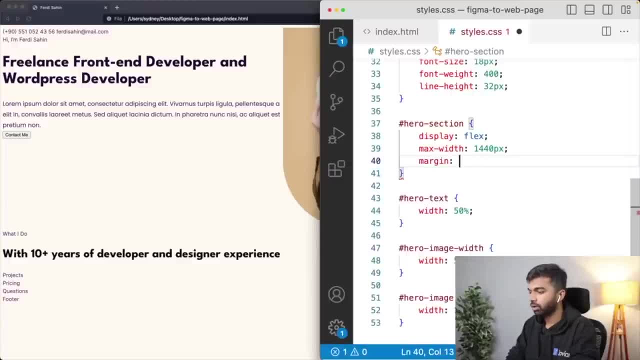 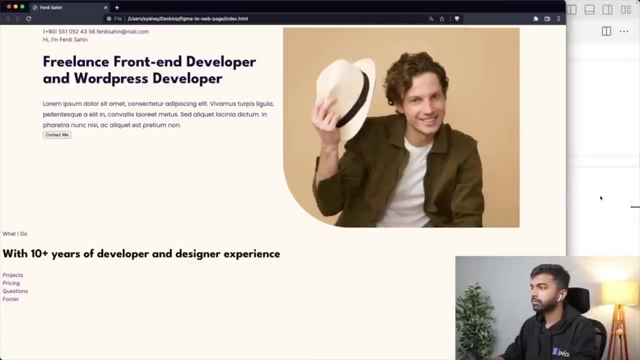 And let me set the margin to zero auto, so that things always remain centered on the page. Okay, All right, So now it's looking a little better. So now we have. now we have this page and on this page we have the on the right. we 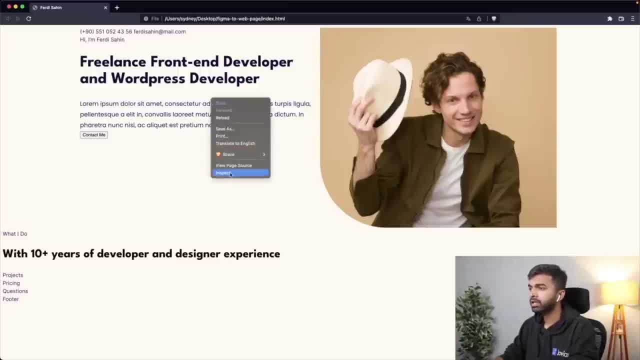 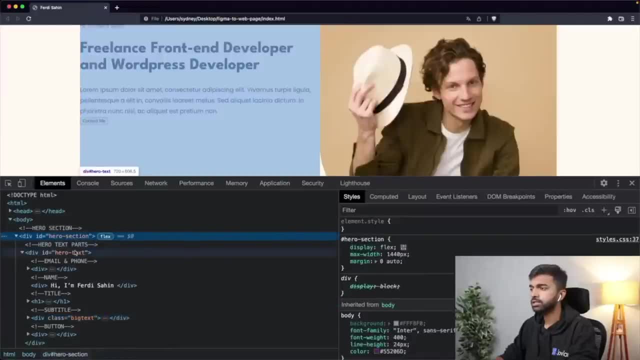 have this hero image. on the left, We have this content And we can verify that both of them are taking up 50% of the space. So here we have the hero section, the hero section. within the hero section, the hero text seems to be taking about about 50% and hero image wrapper seems to be about 50% of 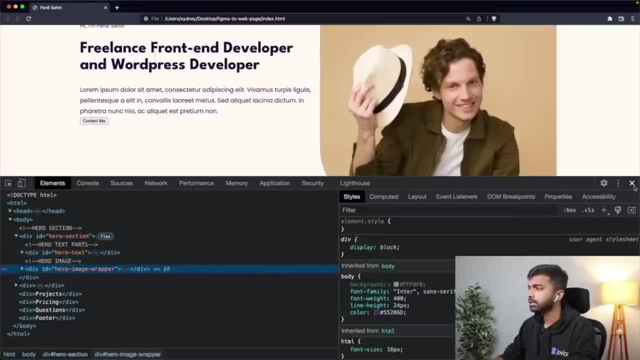 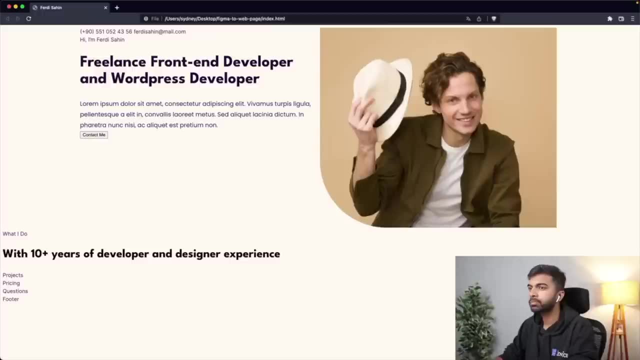 the width, Yep, Great. So now we are getting very close to completing our hero section styles. I can see that there's a small padding or the small spacing here at the top somewhere, So I can probably- that's probably- spacing on the body. 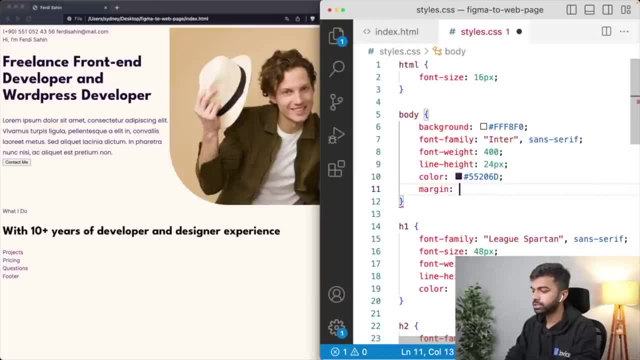 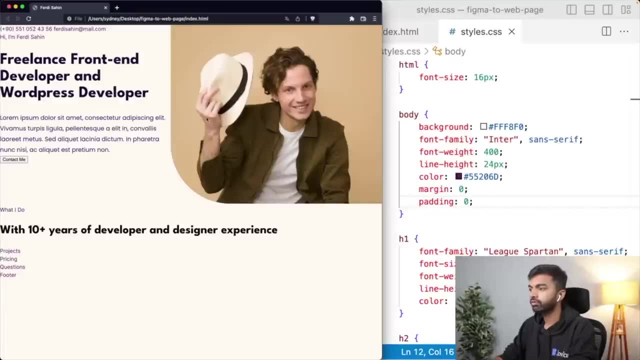 So I may need to reset the Okay So margin to zero and the padding to zero on the body to get rid of that top spacing. Okay, That top spacing is now gone, Perfect, Great. Now let's fix this side. Let's fix the left side of things. 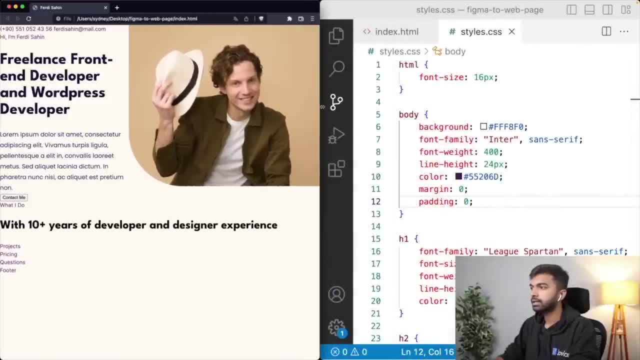 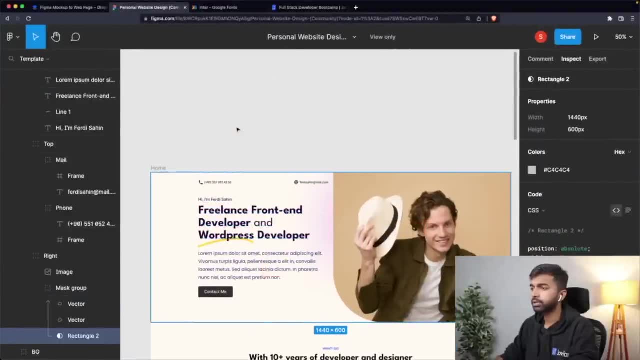 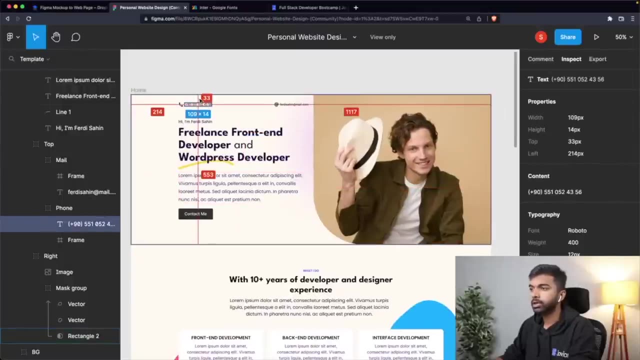 The right side seems to be fine, So let me just bring this back here into half size and let's start actually adding content into this particular section over here, So I can see here that we Okay, So I'm going to. this seems to be about 33 pixels below the top. 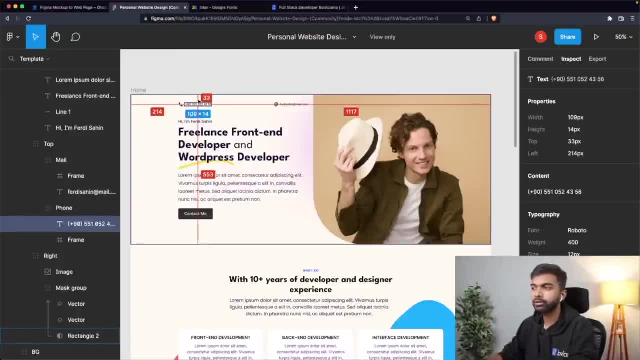 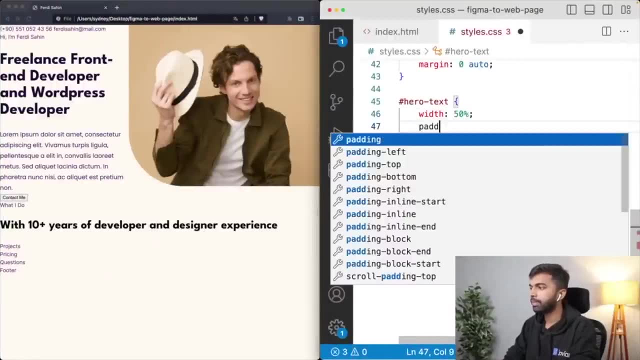 So there seems to be like a padding of 32 pixels. I'm just going to guess about 32 pixels, So I'm going to come into the hero text. I'm going to come into hero text and I'm going to add a padding of 32 pixels on the top zero. 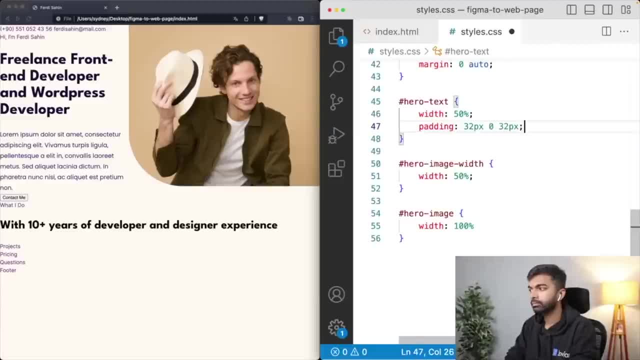 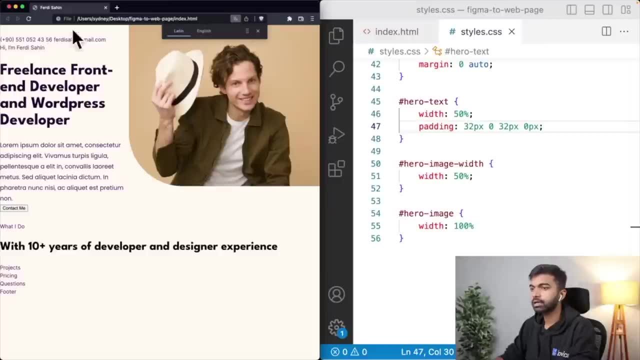 pixels for now on the right, 32 pixels on the bottom and zero pixels on the left. Okay, And let's do that. So now we've added some padding, So things are looking a little bit better. Okay, So that's great. 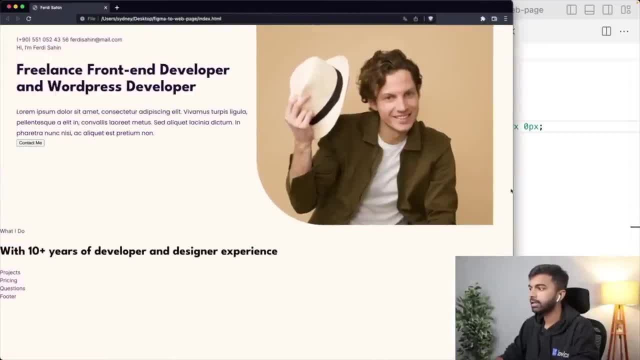 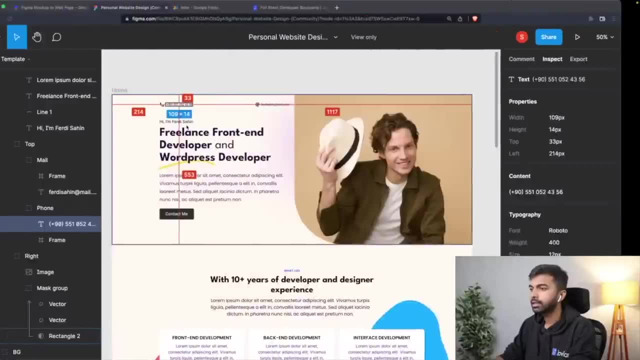 Yeah, So now we've added a pad, now we've added padding. That's good. What next? Well, let's start fixing things one by one. Maybe we need some left and right padding as well. Let's see what left and right padding we can add. 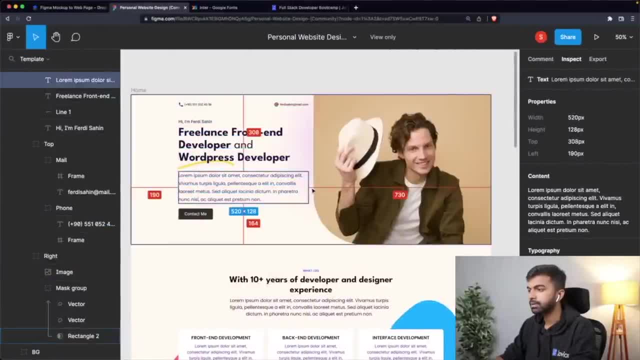 So here it seems to be. there seems to be about a 20 pixel space, but between the text here and the image here, I would probably take a similar 20 pixel padding on the left as well. So I'm just going to make this 20 PX. 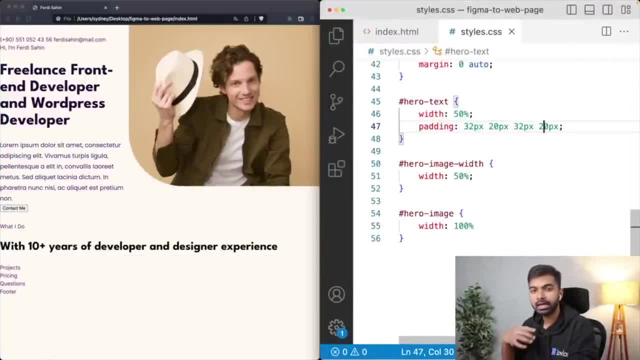 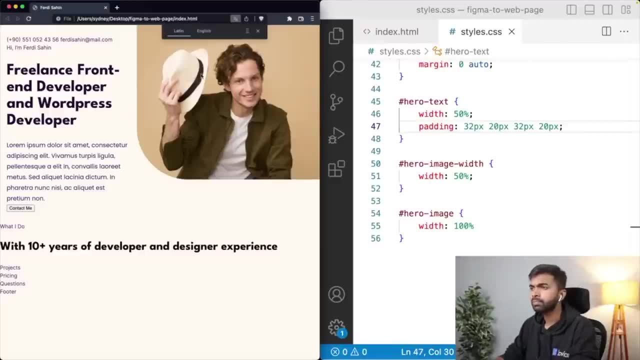 Okay, So these are places where often you may not be able to get exact details from Figma and you may either have to guess or you may simply have to ask the designer. Okay, great, So now we have about. now we have padding. 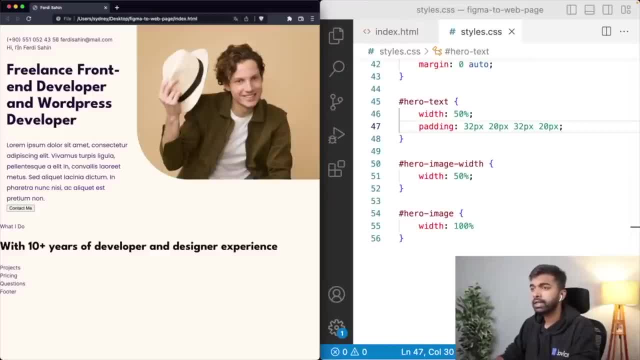 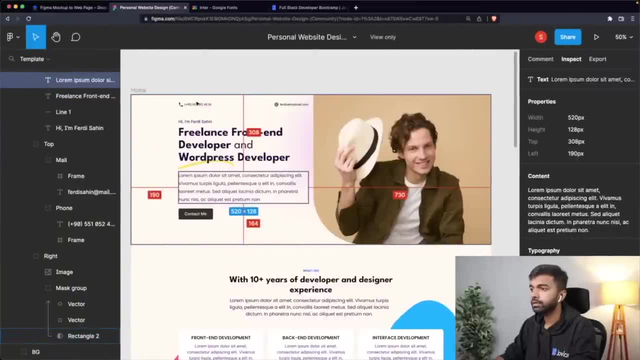 So now things are looking a little nicer. Then let's start fixing one by one things, starting from the top. Now let's separate out. So here we have the phone number on the left and the email on the right, So let's separate those out. 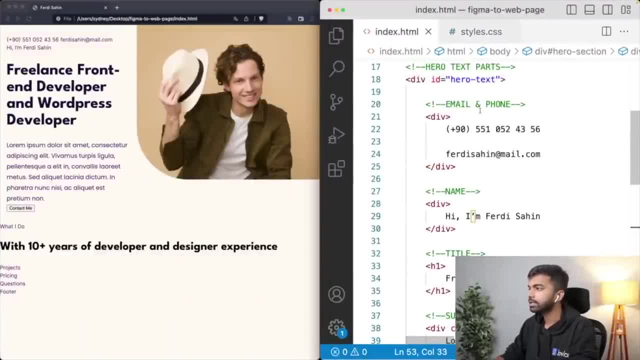 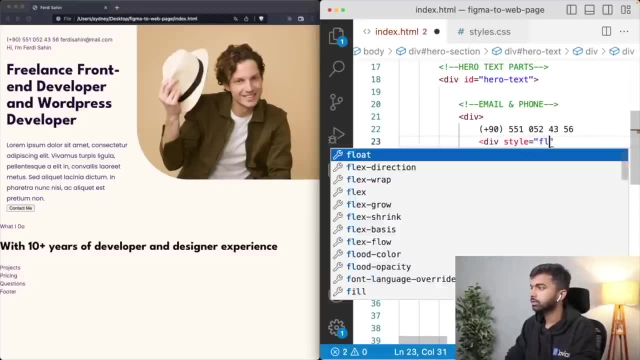 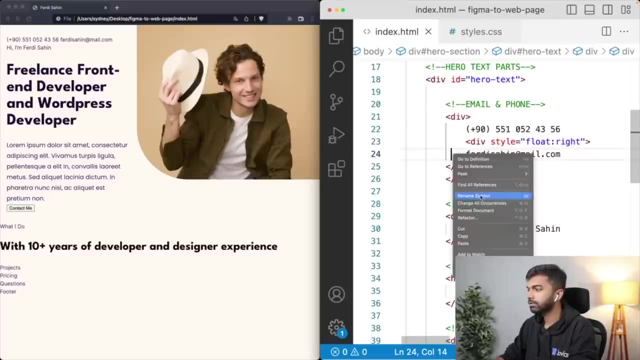 One very simple way to do this, When you have one thing on the left and one thing on the right, is to just use a float. So you could say: div style equals float right, And again, this doesn't always work, depending on the complexity of the situation. 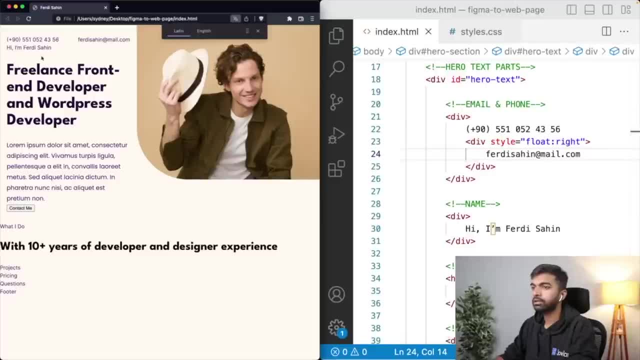 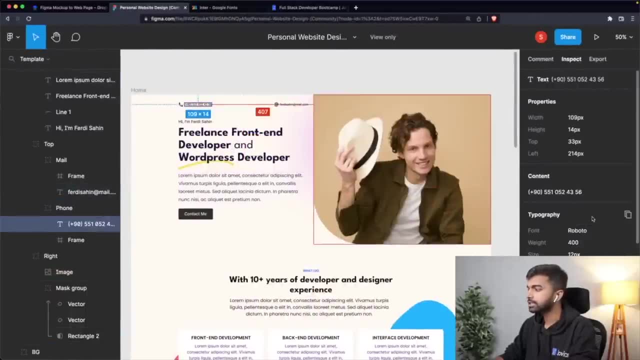 But if you want to do a very simple thing where you want one thing on the left, one thing on the right, that's what you can do. Just use float. So that's fine. Now we've added that information as well, and let's check the font size here. 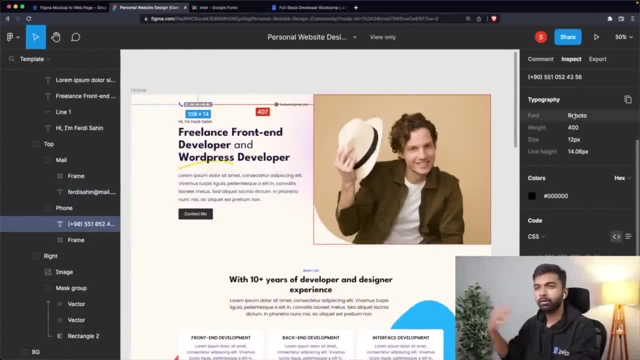 So the font size seems to be small. Again, the font seems to be Roboto- again a fourth font. This seems like too many fonts on the page, So I'm just going to use the font inter for now instead of Roboto, because I don't want. 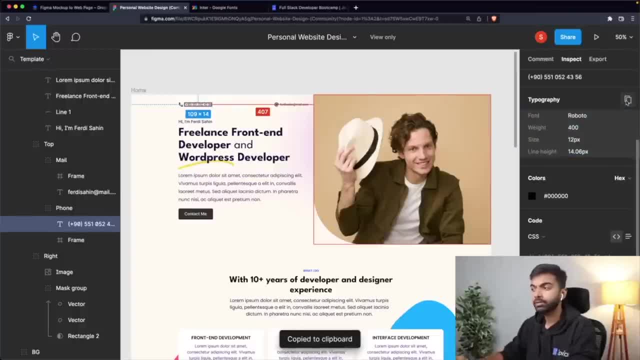 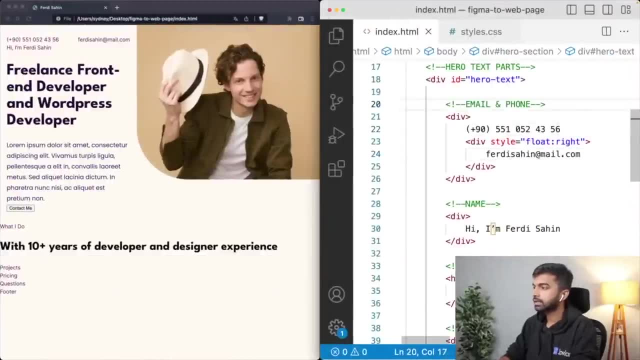 to import another font, and I may need to check with the designer why they have so many fonts, Because three, two to three fonts on a page is generally sufficient. but let us come in here, Let us give this and let us give this a class, or let's give this an ID, because there's only 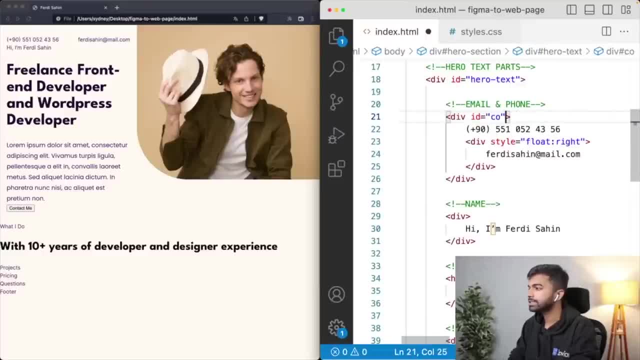 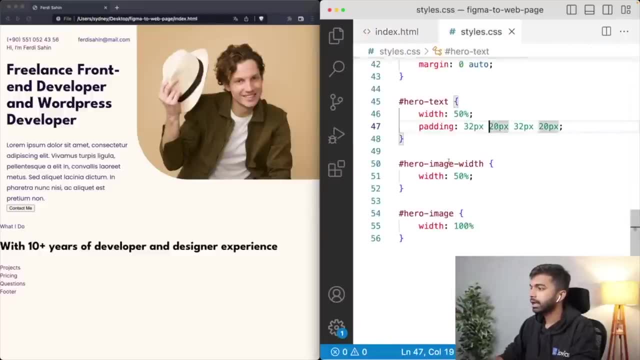 going to be one of these. Well, let us just give it a class code. Okay, This is called small text and we'll use it elsewhere as well. Small text- Okay, And now we will just pick dot- small text, and let us set the font family to enter. 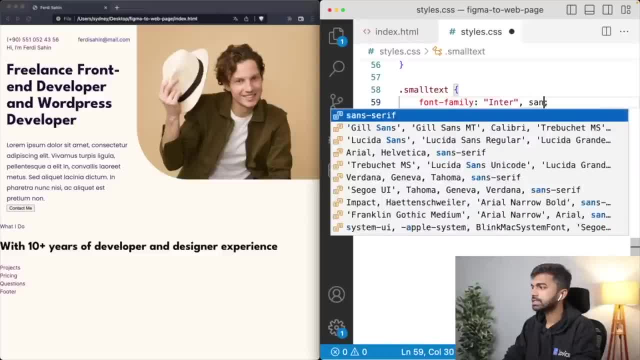 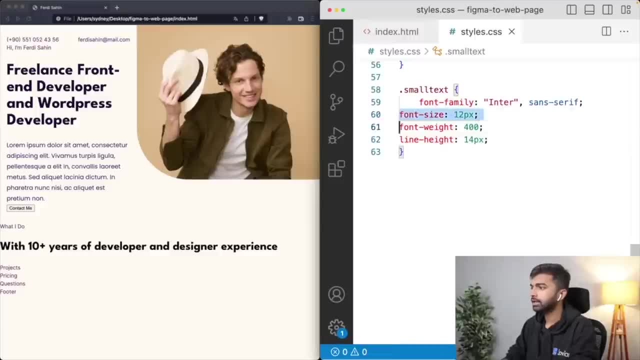 I'm not going to use Roboto here and sans serif font Okay, Line height, et cetera. all that is fine, And I may need to check the color as well. Maybe there might be some change required in the color, but now it is smaller. 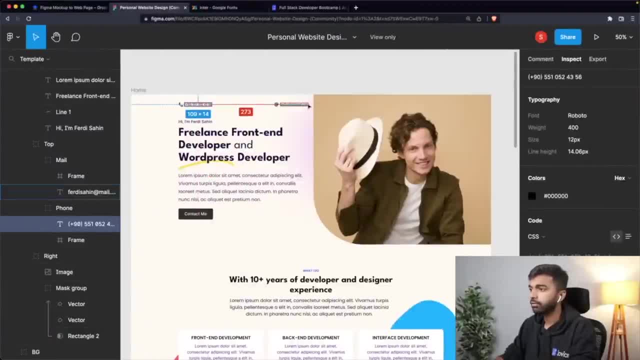 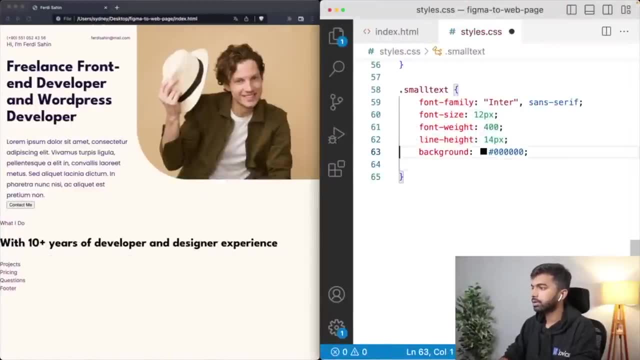 So it's definitely what we are going for. Definitely smaller than what we have. Okay, The color seems to be just black. So zero, zero, zero. So I'm just going to set the color to it. copies as background, but it should actually. 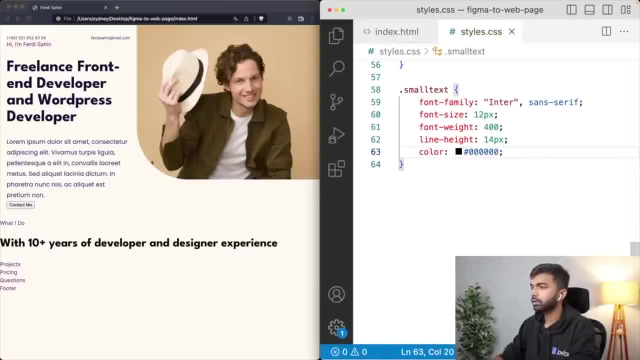 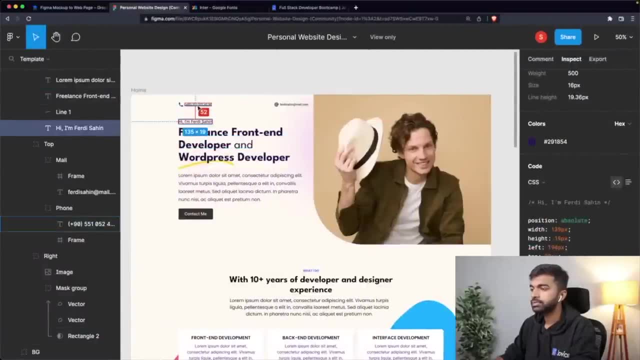 be color. Okay So, yeah. So now the color is fixed and this is all good. Then we have this next section, and there seems to be about a 52 pixels of gap. Normally, these gaps should be multiples of four on, like four, 16.. 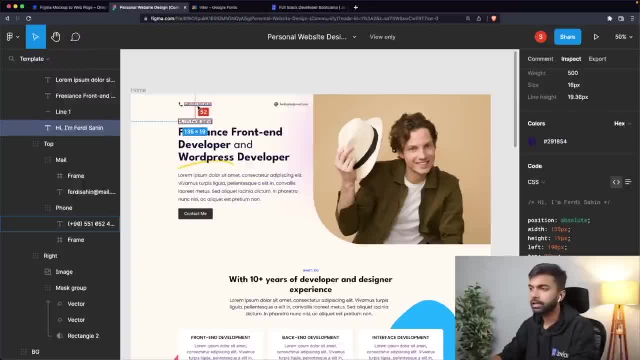 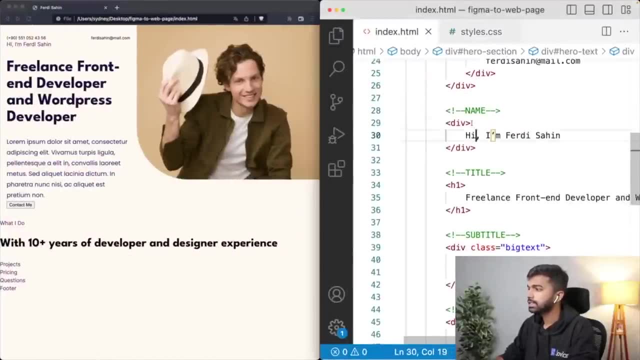 Um 32, 48, but 52 seems to be what they're using here, So I'll just use 52, as per the design. So let me go in here and this is like: let me give this the or, let me give this a small. 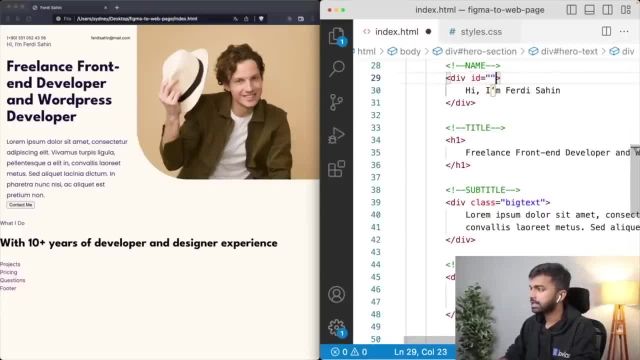 um, let me give this an ID and let's give it the ID name, uh, or like hi And name. So always coming up with good names always hard, but uh always try to give a descriptive name so that when you're just browsing through the CSS file, you know exactly what you are. 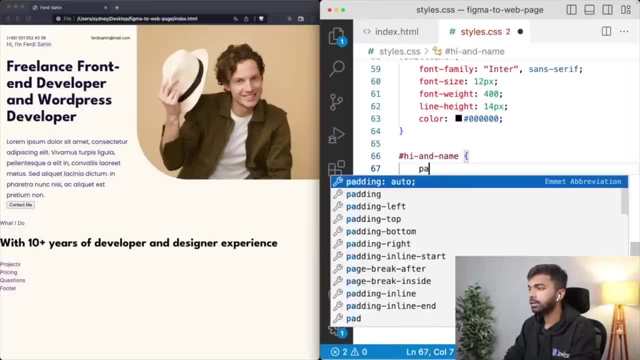 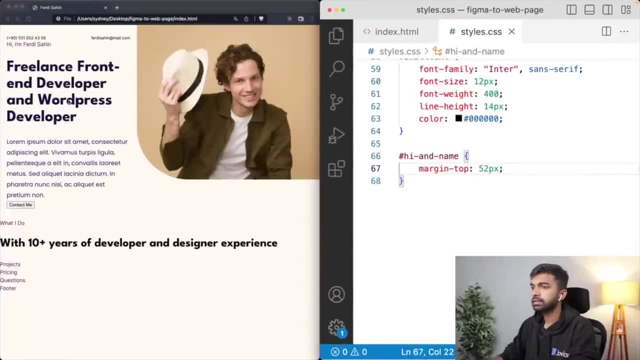 referring to So high end name. right, High end name has a margin top of 52 PX, So let me add that. So now you should see here that there's a margin top of 52 PX. All right, This is. this is good. 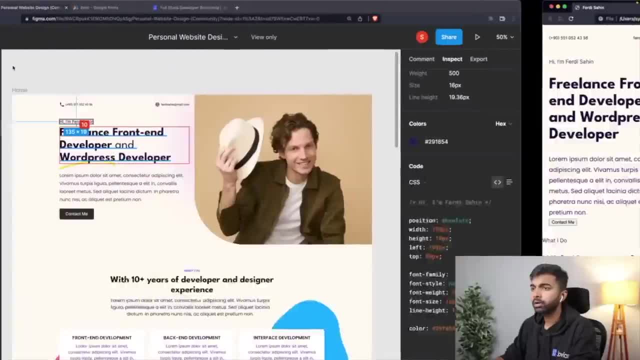 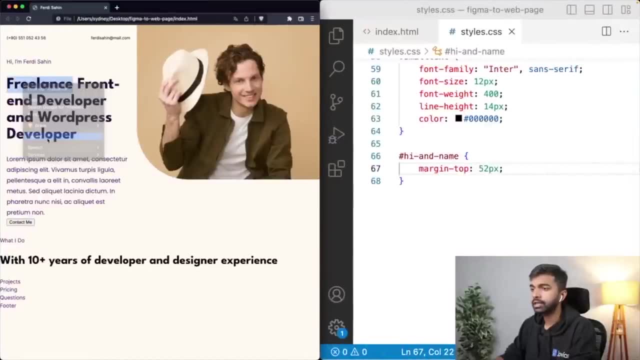 Um then let's also maybe check over here What's going on. We may need too much gap here. The gap here is only 10 pixels. We may need somehow. this gap seems to be higher than 10 pixels, So I'm just going to check here. 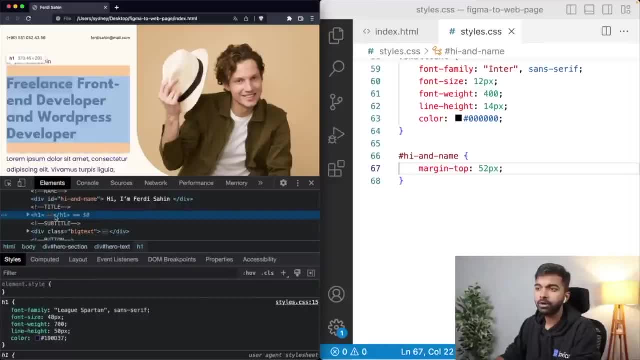 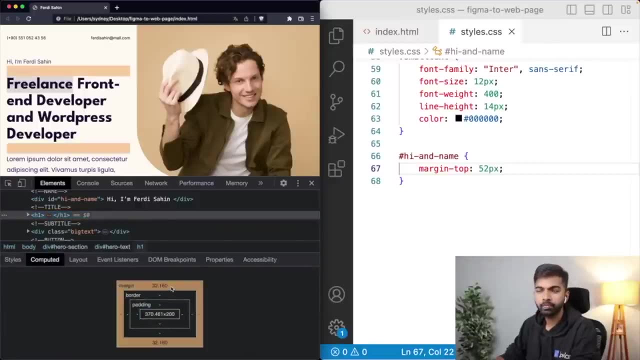 Okay, It looks like this is the default. This is the default padding or the default margin for each one, And right now, the margin- the default margin for each one- seems to be set to about 32, but the default margin that we want is 10 pixels. 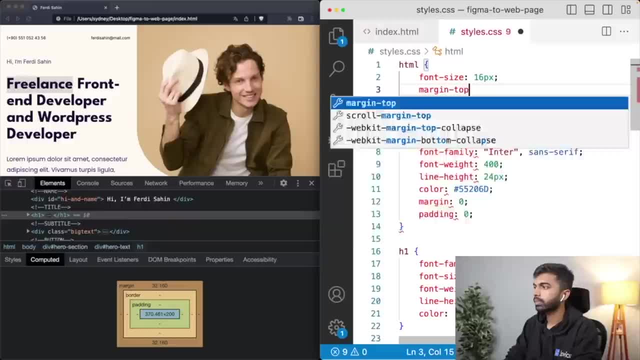 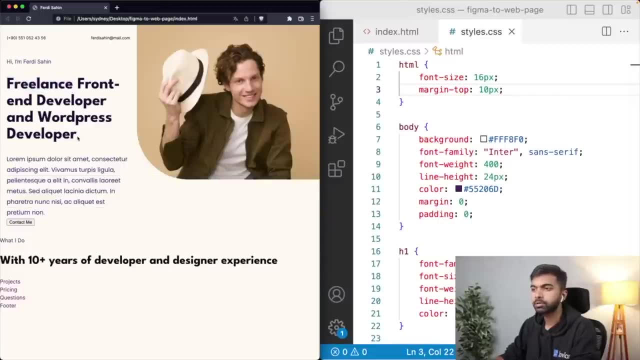 So I'm just going to set this to margin top 10 PX And let me reload that. By the way, I'm using the Inspect element browser tools. This is something that you'll often have to do, Okay, No, sorry. 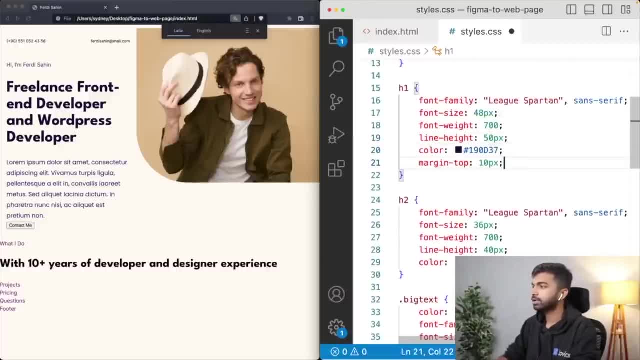 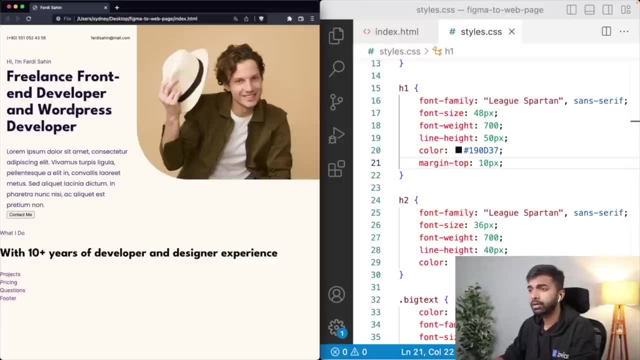 That's not for H1.. That's for and that's not for HTML. That's for H1. margin top 10 PX: Perfect, Great, This is looking fine too. Hi, I'm Fardhi Sahin, a freelance front-end developer and WordPress developer. 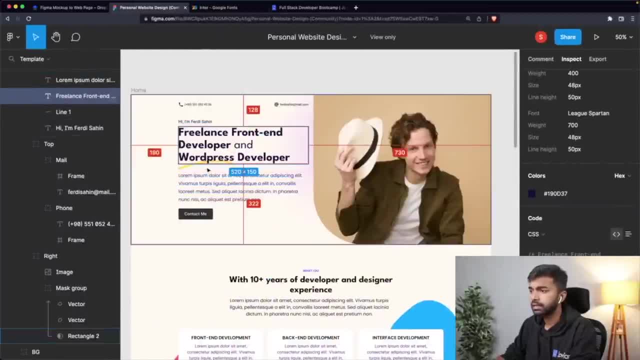 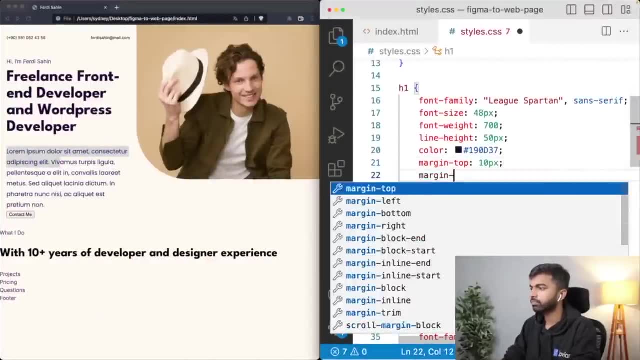 What next? Lorem Ipsum: Okay, This again. the gap here seems to be 30. It's currently 32.. Let's change the margin bottom as well. Okay, Perfect. So I'm going to set it to 30 PX to match the design. 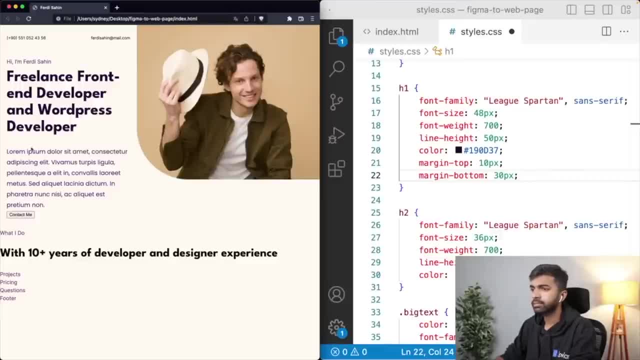 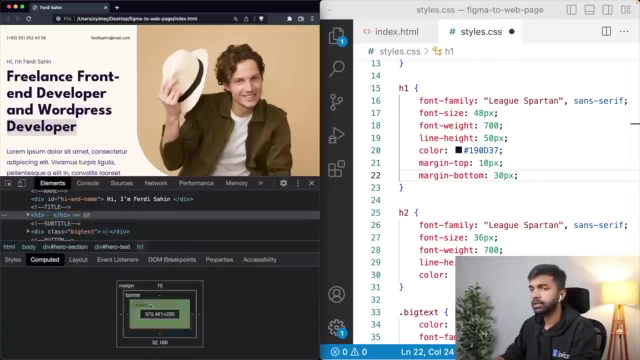 Exactly, Okay, Looks fine. I think we have probably fixed the margin here and we can always verify by going into inspect element. So we go into inspect element, check the computed settings. They can check that. Okay, Margin bottom seems to be 32 still. 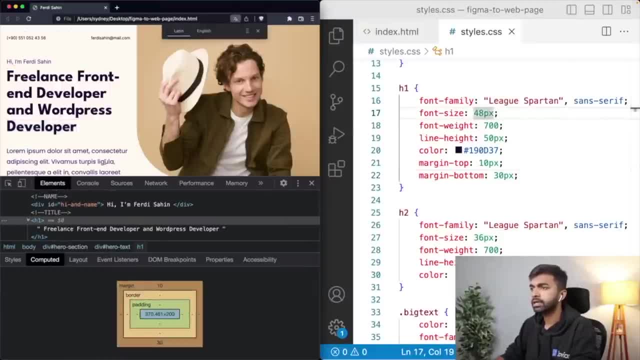 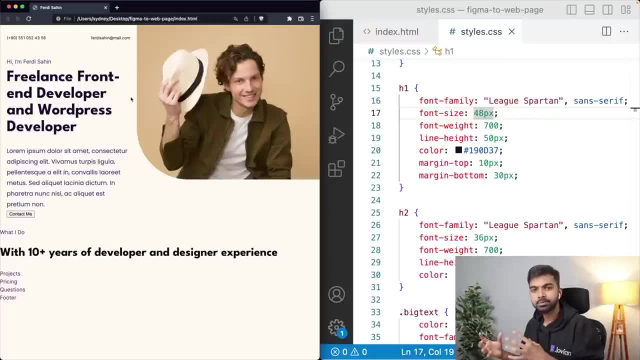 Oh, I'm not saved it. Yeah, So now it's a little closer, It's a little better. So this is what you do. You look at the design. Okay, You go to the HTML file and add some CSS properties. 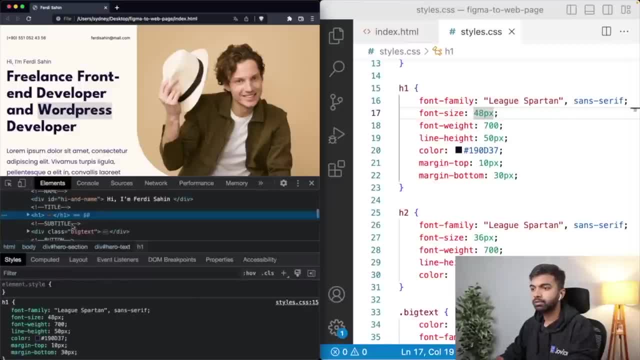 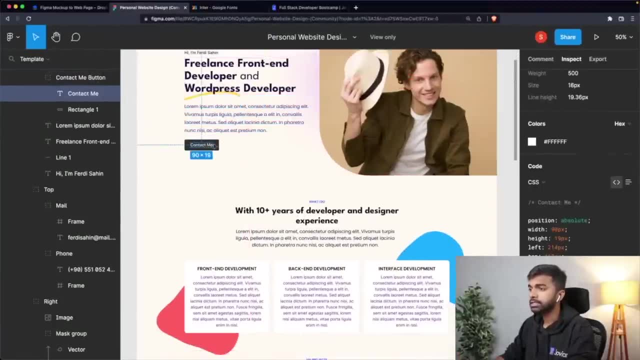 Then you go and inspect to make sure that things are exactly as you want them to be, All right. So that's fine. What next? Well, we have this contact button. Let's try and fix the color, and the font is, et cetera, for this button. 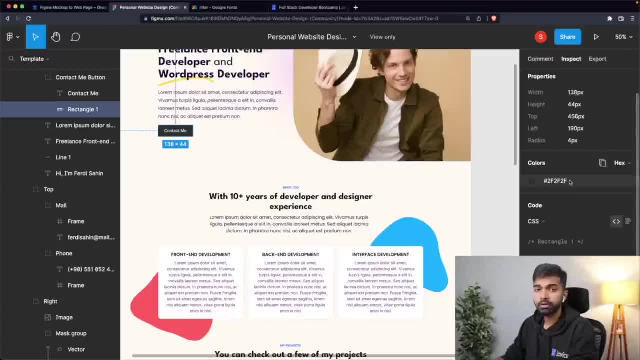 Okay, So the background color seems to be 2F, 2F, 2F. So that's what I'm going to use for the background. And then the width and height also seem to be provided here, So width is 44.. 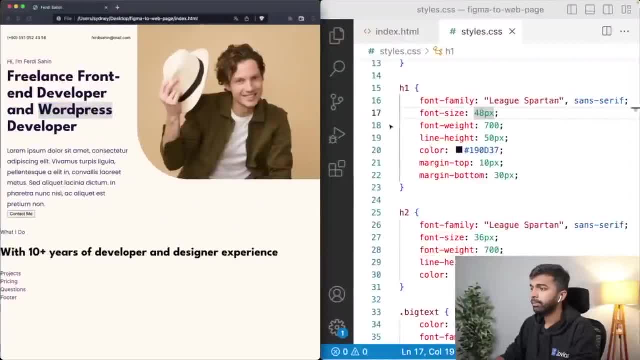 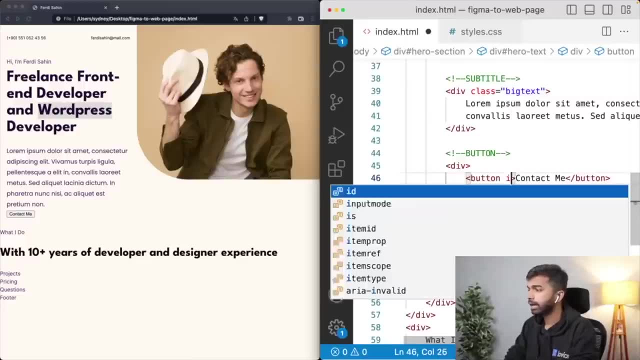 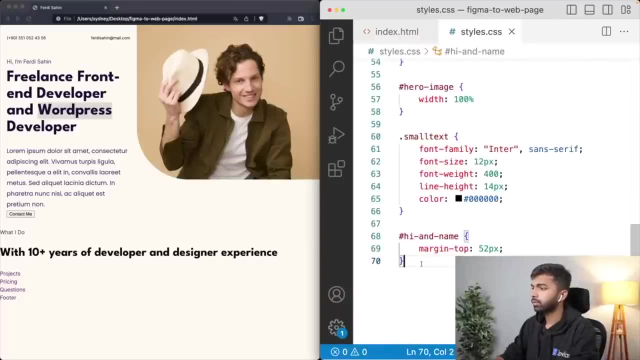 Let's just copy them all And let me come back here and let's go into the button here and let's give this a. let's give this button a ID. Let's call it contact button. Let's come in here, back into and let's paste in all the properties. 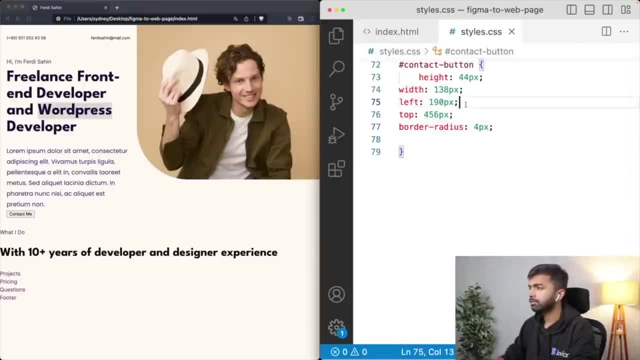 So we are adding a height, We are adding a width, We are adding a left. I don't think we need this left and top, Generally speaking, because we are already arranging things in the right order, So we won't need that. 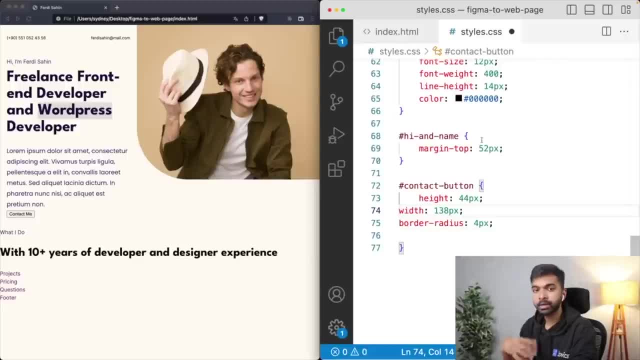 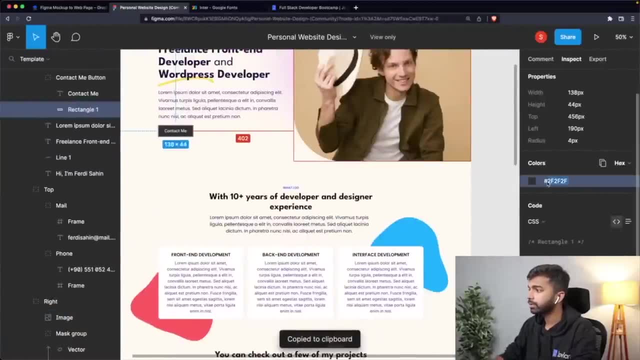 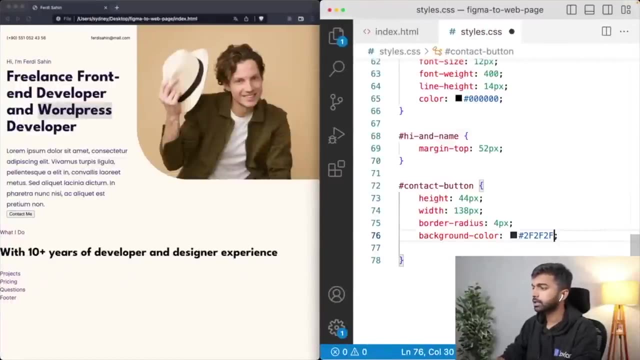 So that's why be wary of copying things directly from Figma. Sometimes you might get weird results. but width and height is something that I can use and I can add a background, So let me grab the background color as well. So let's see background color: 2F, 2F, 2F seems to be the color that we're using and looks. 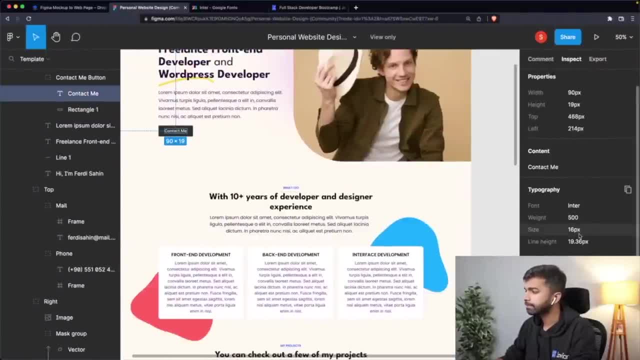 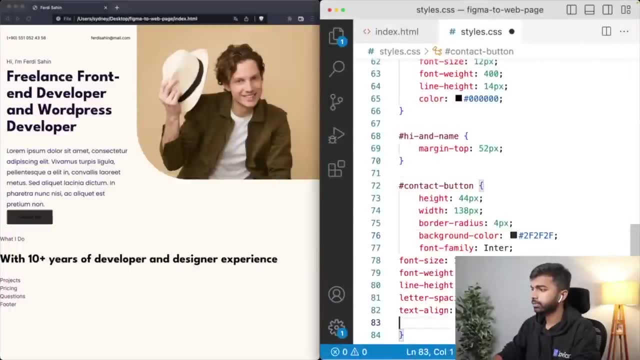 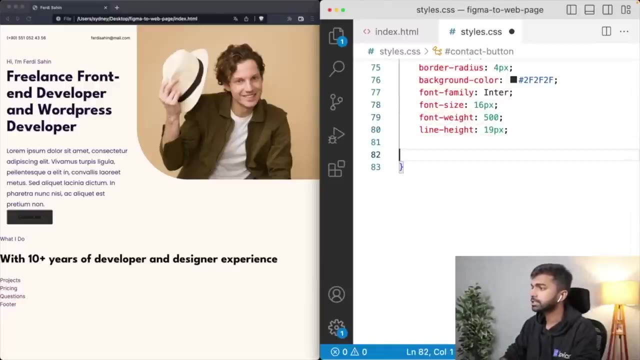 like the text color also needs to be changed. So the text color In this case, well, the text size is 16 pixels, The line height is 19.. Let me just grab that and put that in here. Font family: inter font size is: font weight is 500, line height is 19, font size is 16 pixels. 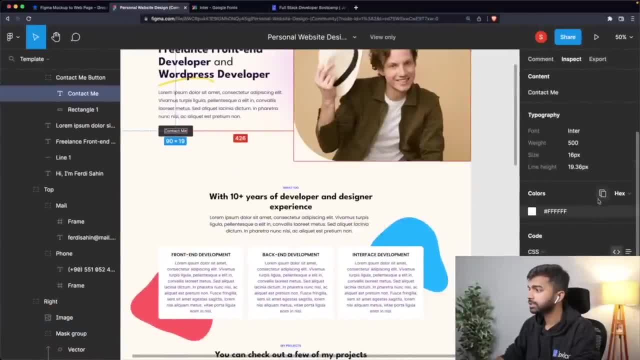 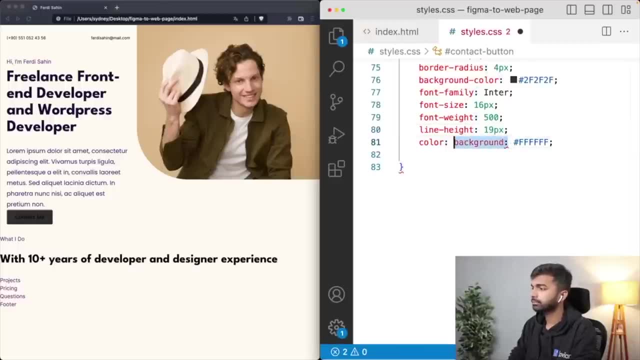 Okay, And there's a text color as well. The text color just seems to be white: FF, FF, FF. So color is just going to be Ken, All right, Okay, Okay, Okay, All right, And there is some space above this. 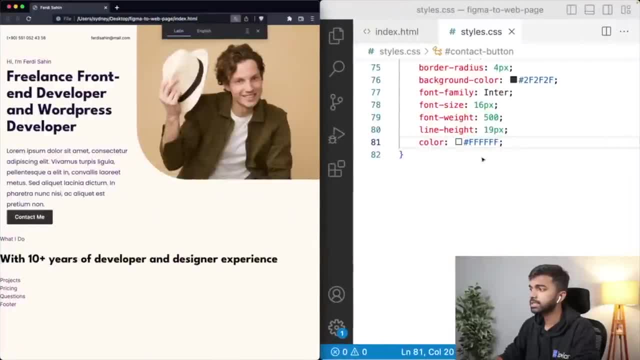 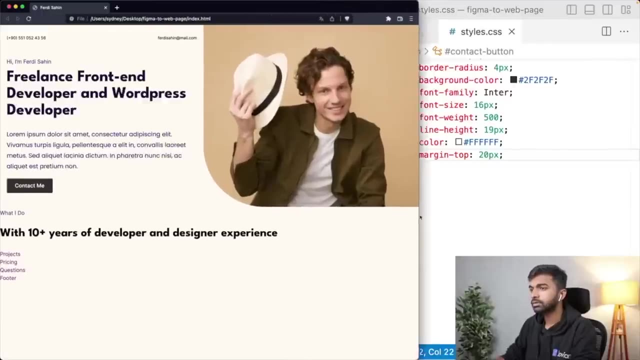 So this about. there's about 20 pixels of space above it, So I'm just going to say margin top 20 pixels. All right, Okay, So our hero section is looking good. Now I'm not going to get into responsive design in this particular tutorial, because now you 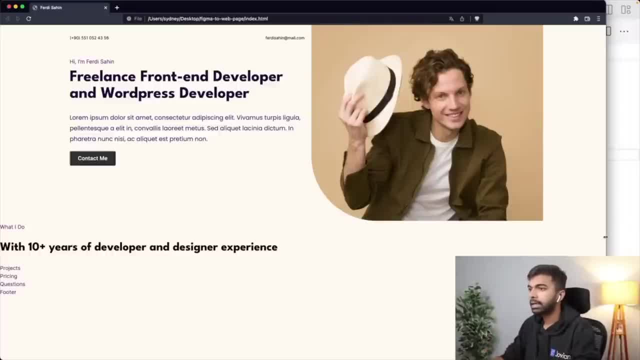 may ask: okay, what, how does it look like on mobile, et cetera? But at the very least, if I compare it to what I have here, I think this is looking fairly similar. Hi, I'm Ferdy Sahin. freelance front end web developer. WordPress web developer. a subtitle. 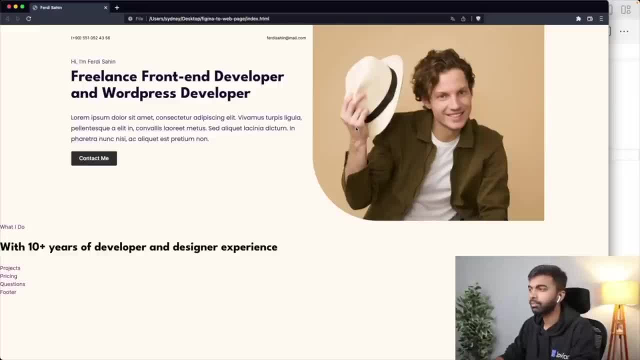 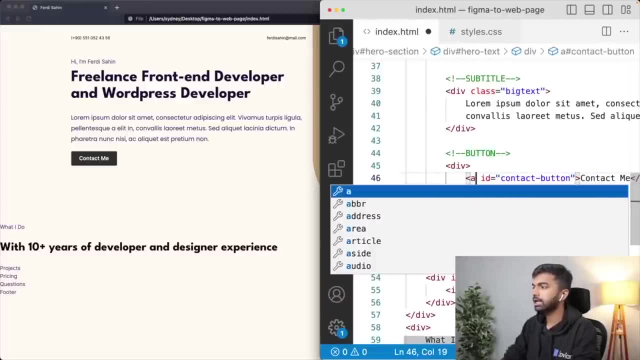 and then a contact me button, and clicking on the button may probably open an email or something like that. So let's actually just make the button functional. instead of the button. I'm just going to use an A tag and I'm going to put in a mail to link so that clicking 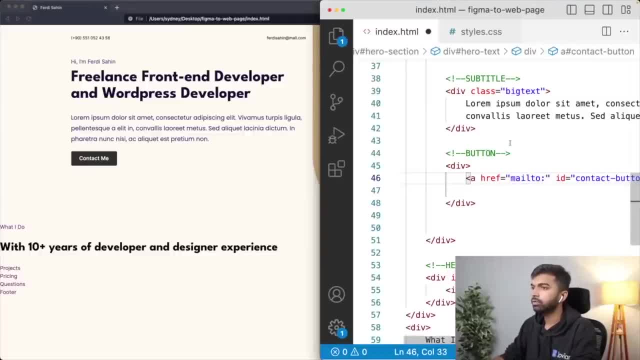 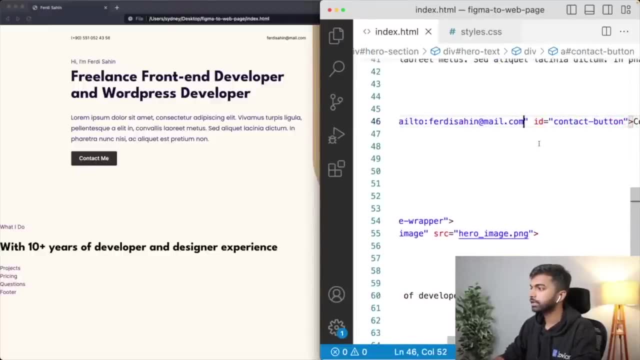 on, it will open up mail, Okay, Okay. So I'm going to mail to Ferdy Sahin at mailcom, So let me, let me just grab that and let me put that in here and let's just say: target equals underscore blank. 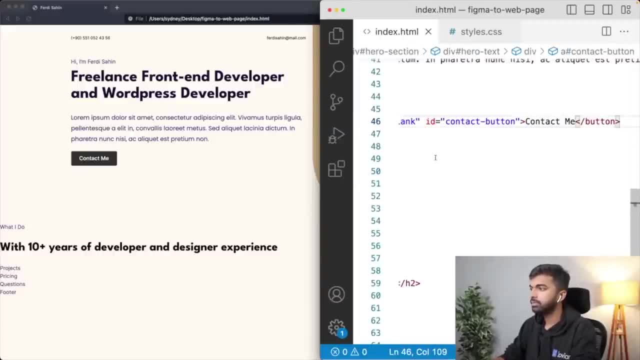 Okay, So that's going to open up email thing And I think we don't need this div at this point. So whenever you feel that a div is not necessary, you can always just go ahead and delete that div. Okay, Let's come back and let us change that to slash a. 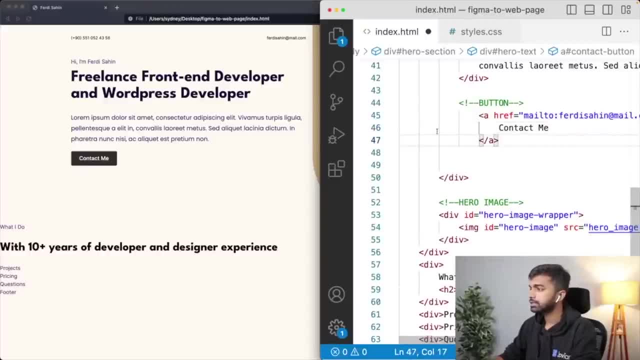 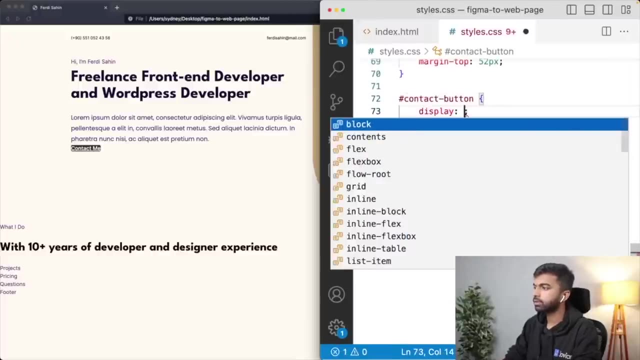 Okay, And let us just format the document and save it. Okay, That's not doing it. Well, I think eight tags. you might also need to set display block for eight tags in case you want to add margin and padding. Okay. 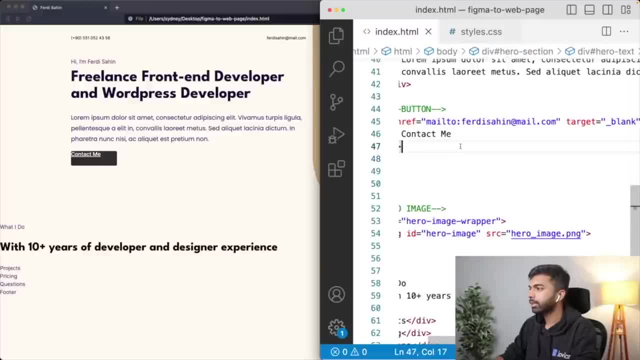 I'm still not doing it. I'm just going to, I'm just going to keep it to a button for now. Let's forget that, Right? So you have to sometimes make these decisions. What should be? which kind of a tag? 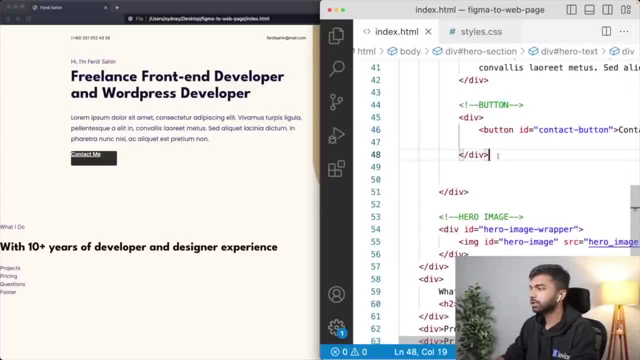 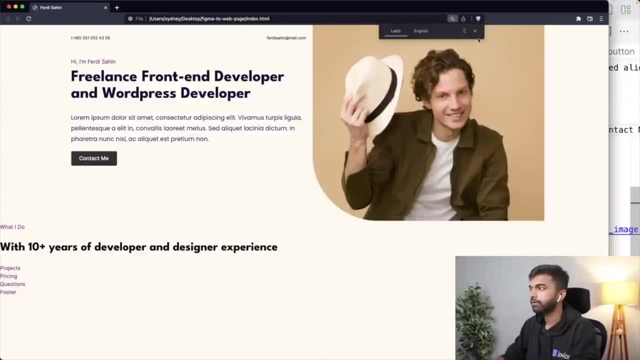 In most likelihood, you will probably be just using a framework that will take care of these things for you, But for now I think let's just keep this button, which is not exactly functional. So with that we are more or less done with the hero section. 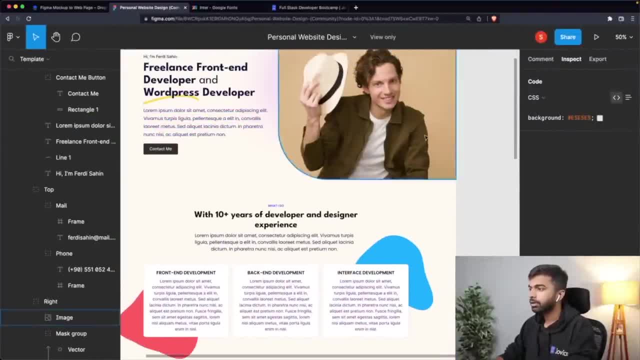 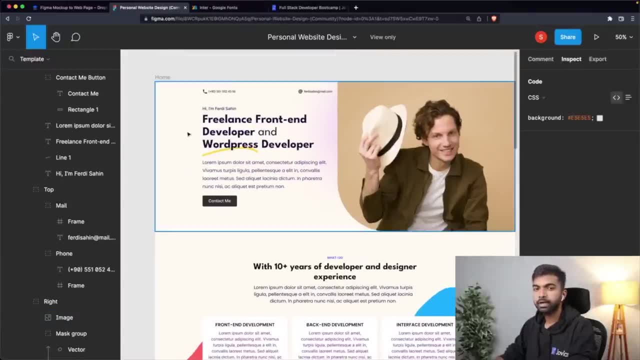 You might notice that in the hero section, our content here, our image, actually goes all the way to the right, but the text does not go all the way to the left. So we may need to fix that, So. So that is what I mean by saying: do the easy parts first. 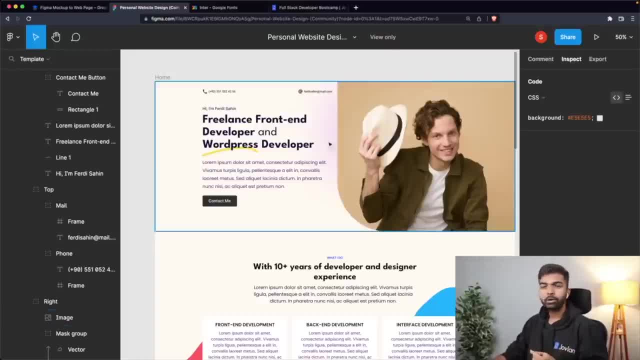 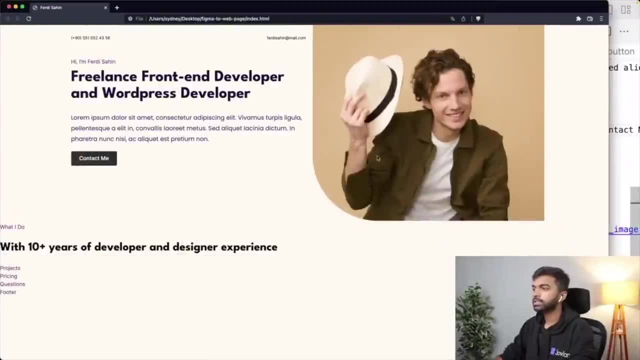 What do you might want to do is implement the entire page and then figure it out exactly how you're going to implement this behavior, because you also have to think about what happens when you resize the page and all in in this case. for now, I'm just going to keep. 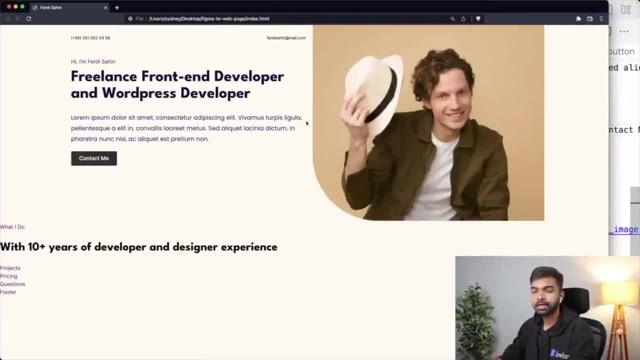 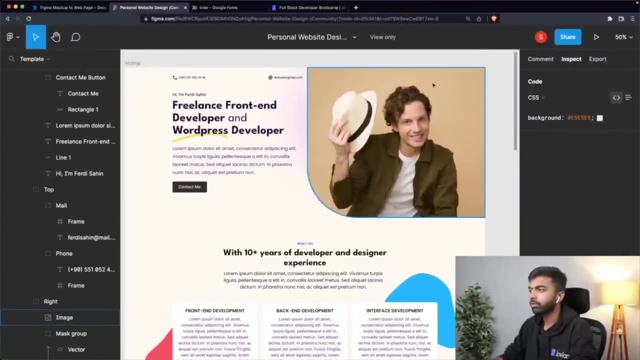 things equal with for now and I'm going to come back and maybe fix it later when I have the time, Okay, Or I'm going to go back to the designer and say, Hey, this design looks a little odd because over here it kind of goes all the way till the end over here. 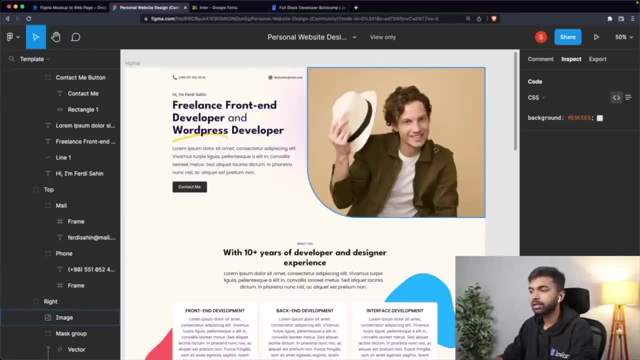 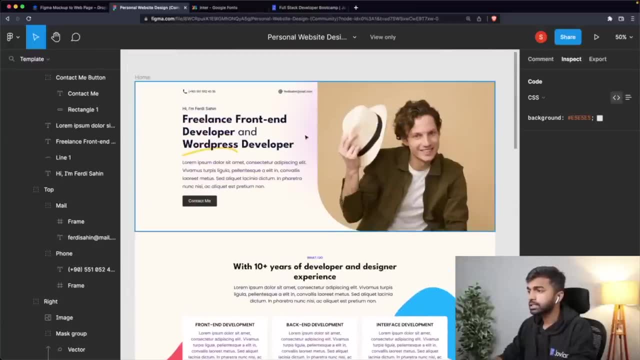 It doesn't. How about we keep it centered on the page? Okay, And how about we make sure that all the content is centered on the page so that we don't run into these issues? Okay, So that is a hero section. There's also this thing here in the, in the background. I'm yeah, I'm not sure how exactly. 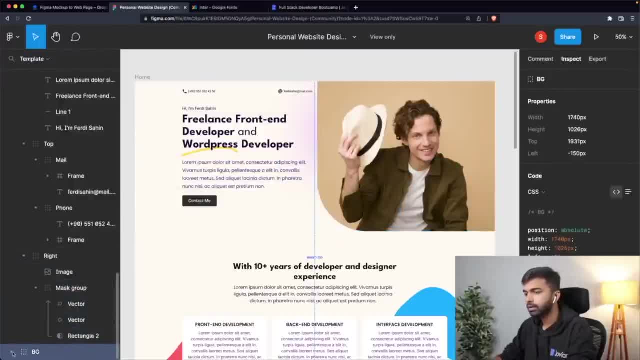 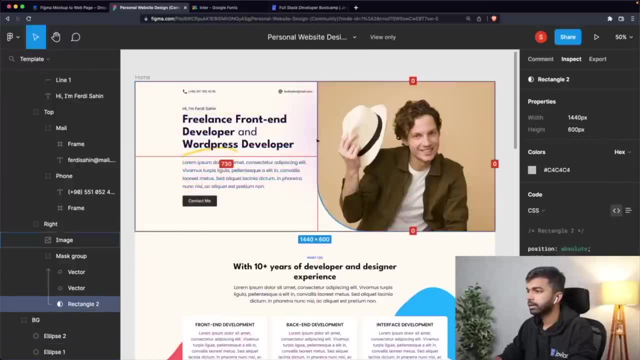 we can implement something like this. Let's see, in the background we have this ellipse of some kind. Okay, We'd have to figure it out. Okay, We'd have to figure out how to add this glow. It may not even be that easily possible. 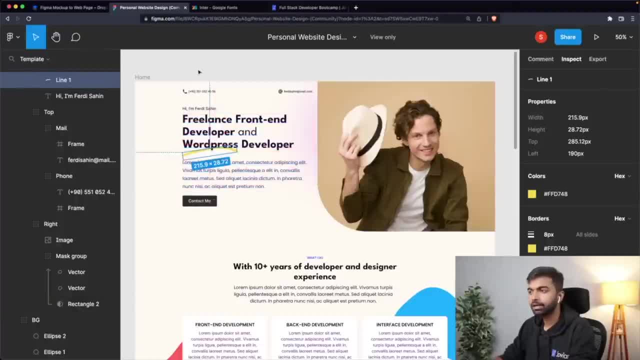 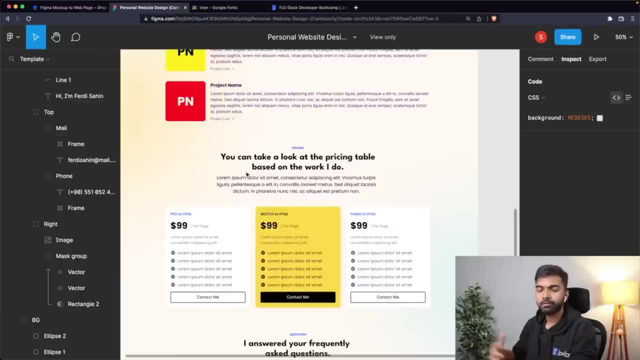 And we'd have to figure out how to add this image, And again, that is something that we can possibly look at towards the end, or something. Okay, Cool. Well, I think we'll do one more section, because we can, of course, as we keep doing this. 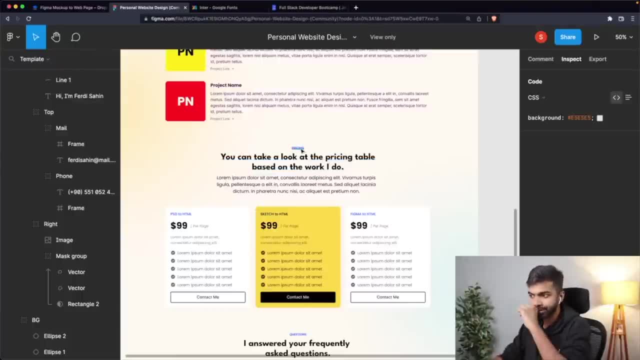 is going to take a lot of time. So how about we do one more section? let's do the pricing section and I leave the other sections to you as an exercise. So let me come back here and let me get rid of- uh, let me get rid of these other sections. 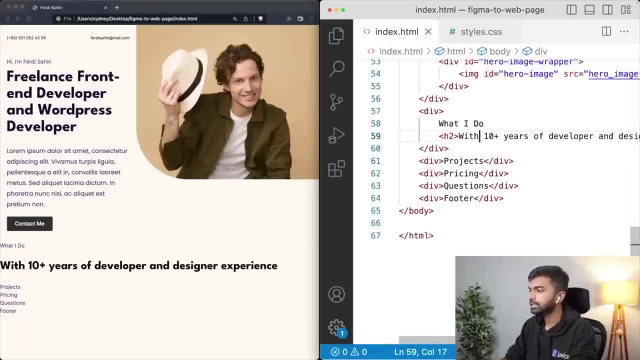 Okay, Okay. So let me get rid of these other sections. So I have this what I do, section that is left as an exercise. I'm getting rid of that. By the way, you can comment out an entire section like this: 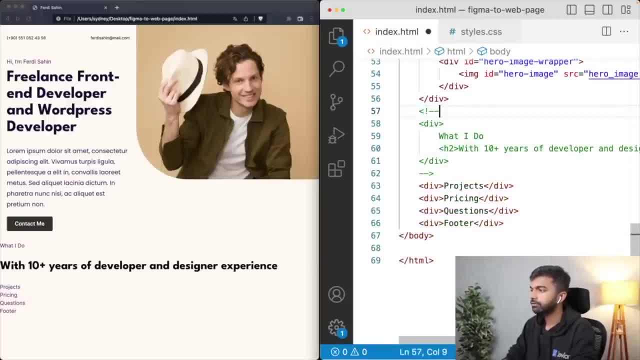 So just start with exclamation mark, hyphen, hyphen, and close with hyphen, hyphen, exclamation mark, And then that way you can comment out an entire section. Let me do that, And let me do that with projects as well. 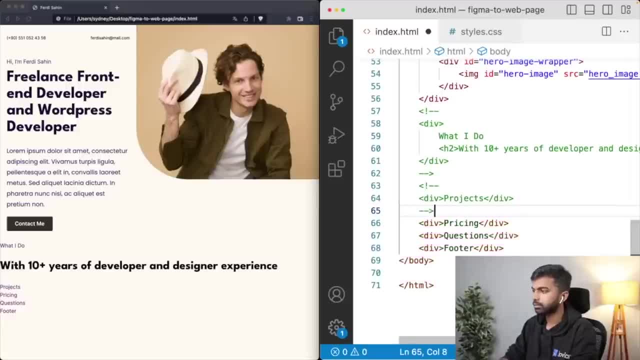 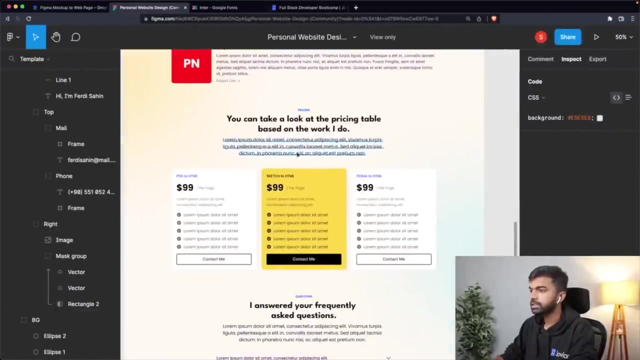 Let me just comment that out. for now I'm going to implement the pricing section. I'm going to comment out the questions and the footer as well. okay, And let's go ahead. And now let's start implementing the pricing section. So this is the pricing section. 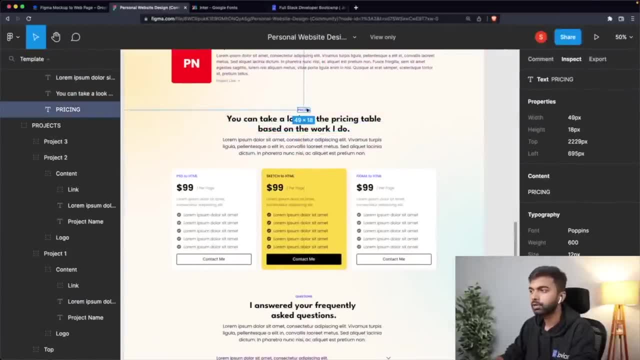 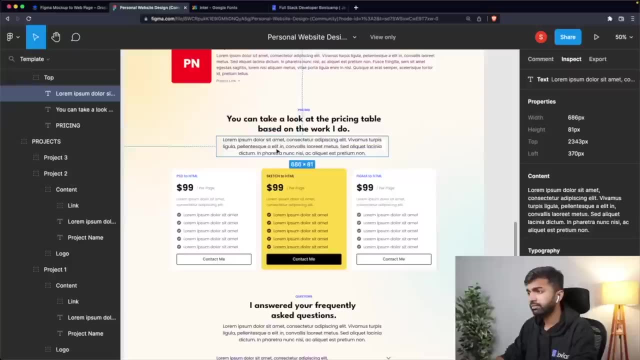 And in this pricing section we have like the small thing here, this blue thing called pricing, and we have, uh like a subtitle or a or a heading, Okay H2.. Then we have this subtitle and then we have a bunch of these boxes. 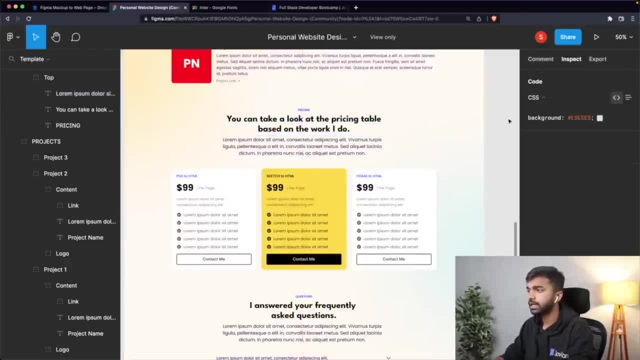 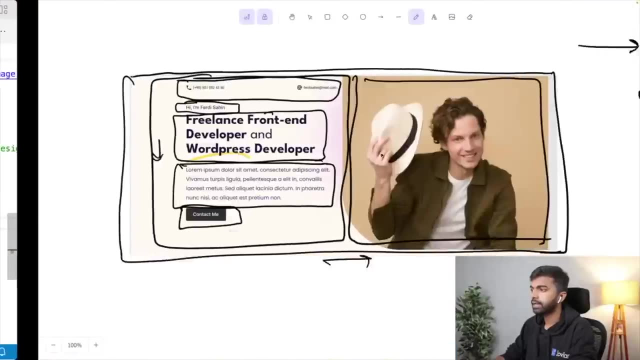 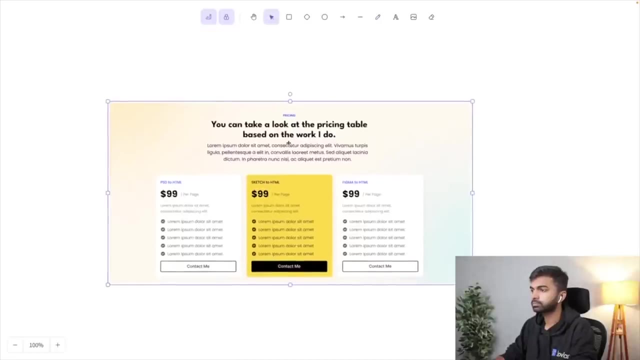 So let's see, let's again go step by step. Let us first take this and create a box around it, Okay, And let's come back here into our oops, our drawing tool, and let's draw some boxes. So in this case, there is 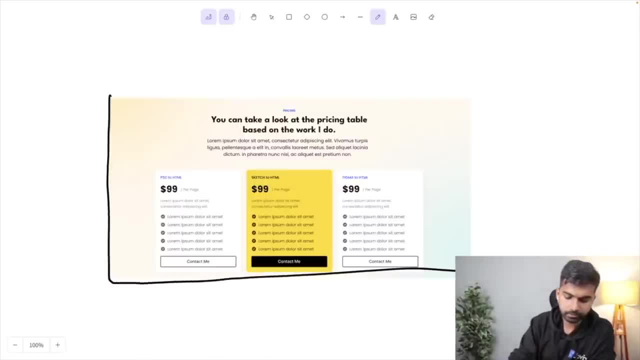 Okay, So in this big box right here- that's where that's what everything is under- in this big box- I can see that the direction of elements is downwards coming down. So there's definitely this one div here at the top which is the pricing. 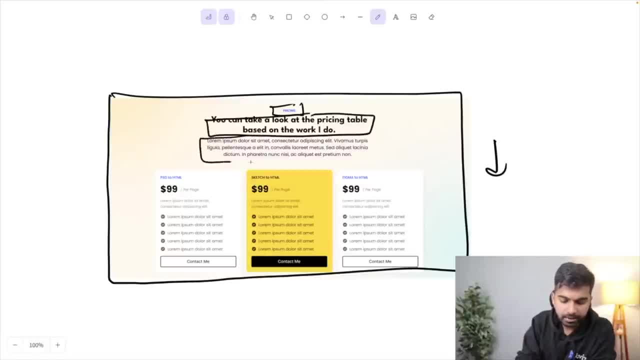 And then there is this other thing here, and then there is this other thing here. So there are three things: pricing- You can take a look at the pricing table based on the work I do in the near that subtitle- And then there is this box that I can draw. 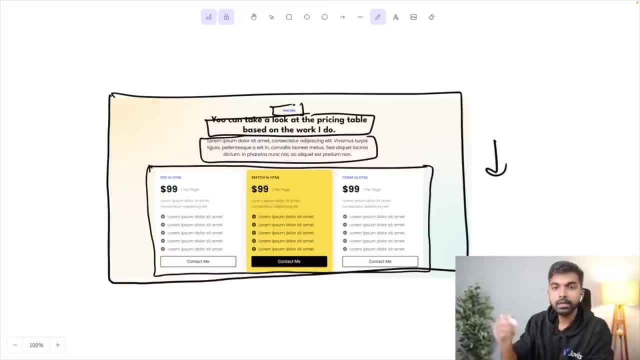 So always try to draw full boxes In that direction. All right, So in the downward direction, in the outer div, we have one, two, three, four boxes. So let's try and achieve this for now, And then we'll go inside this inner box later. 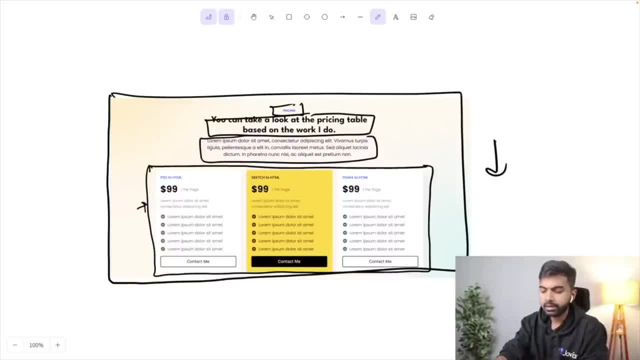 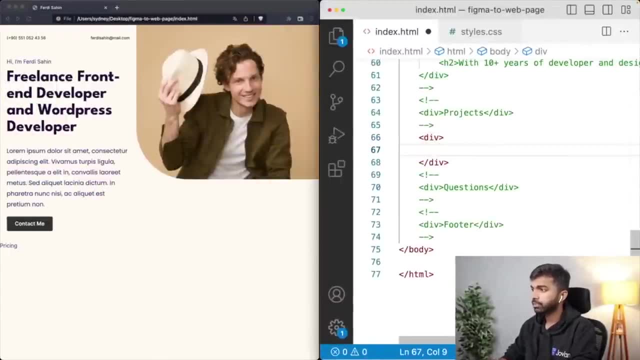 Okay, So I am going to come back now and let's start adding some of this content. So in the pricing section, I just think I need this: the direction is vertical, So I don't need to do display flex or anything like that. 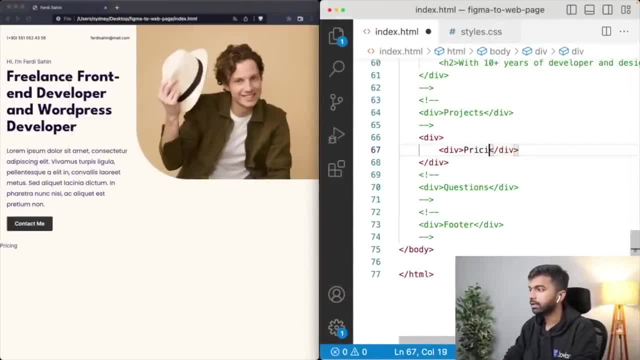 Let me just add: Okay, Okay, So let's add a div here and let's just type it. type out the word pricing. Let's add another div here. Actually, this seems to be an edge too, So we can just use an edge to here, probably. 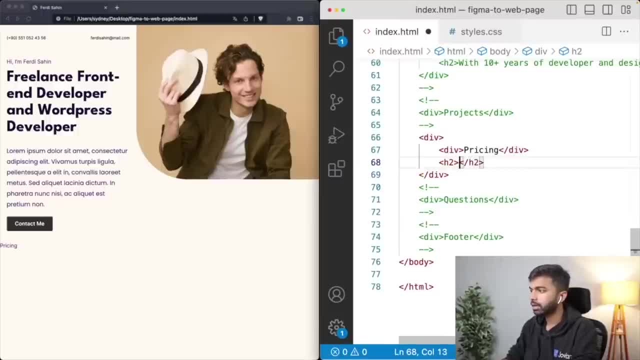 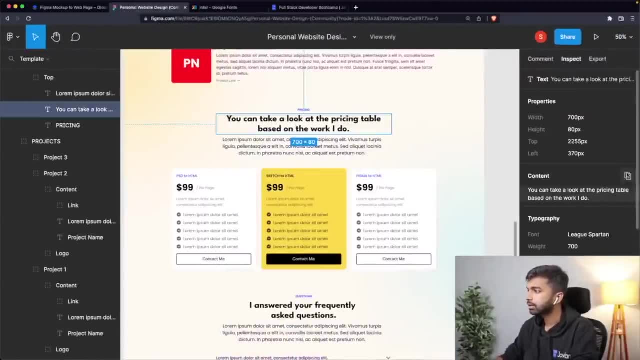 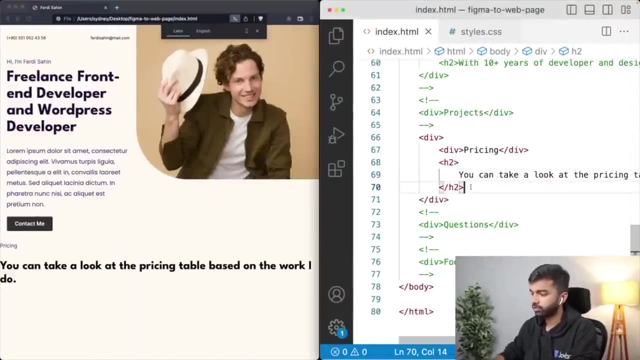 So, edge to edge to, and let's grab this content, which is: you can take a look at what I do, et cetera. So let us just copy and let us paste this content. Okay, It things are starting to take shape. 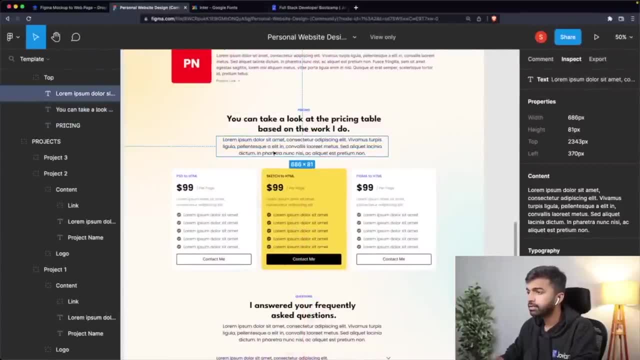 We will come back and fix things a little further. Okay, Then we have this lorem ipsum dollar cell. Okay, This seems to be the description, like a subtitle. I think this seems to be the big text It's about. let's see some. it's 18 pixels. 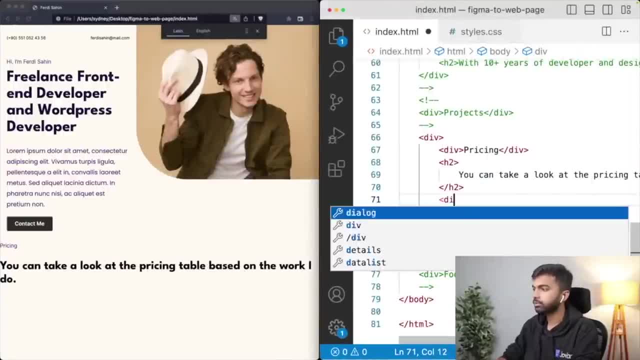 So this seems to be the big text, the same kind of big text that we have here. So I'm going to create a div, I'm going to give it a class of big text and I am going to paste in this content here. 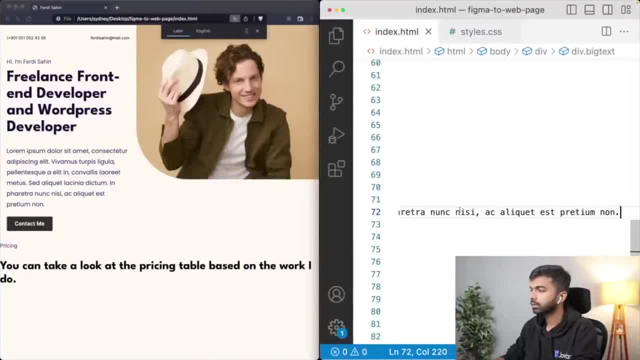 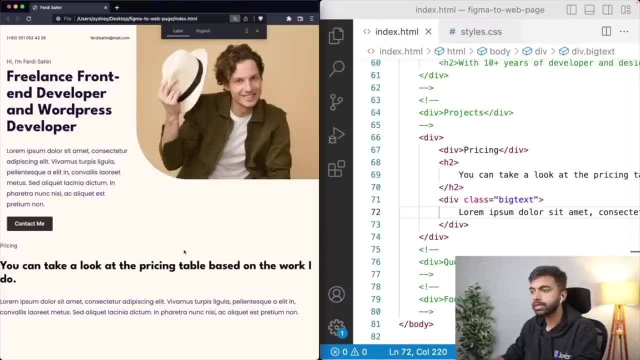 Okay, Okay, Okay, Okay, Okay, Okay, Okay, All right, So now we have pricing, We have this big, we have this header, We have this big text And finally, we have this actual pricing boxes. So for now, I'm just going to create a div and I'm going to say pricing boxes. 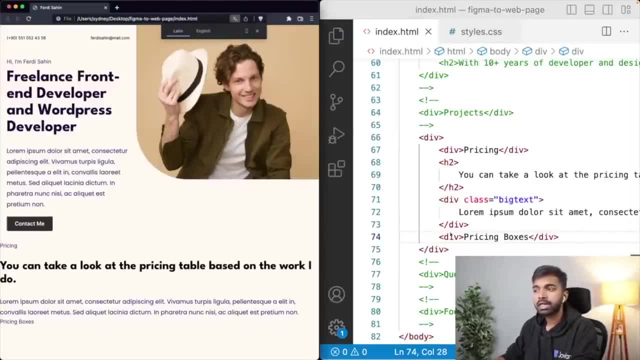 All right, So that's everything that we need to going to put in into the pricing section for now. Now let's start fixing the style one by one. The first thing is that you can see that the pricing section. It's also centered. 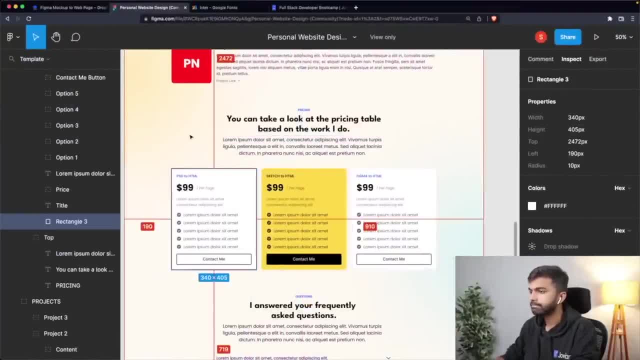 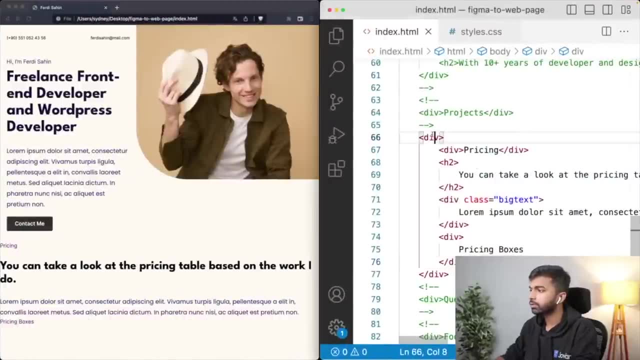 It's a, it's centered on the page and yeah, so I'm just going to give it a maximum width as well. So I'm just going to go into the pricing section. I'm going to say: ID equals pricing section And what is the idea of the pricing? 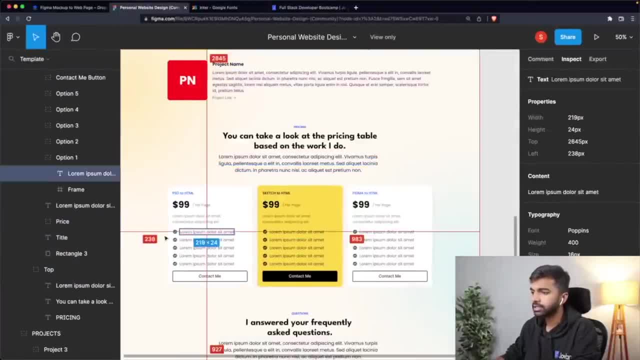 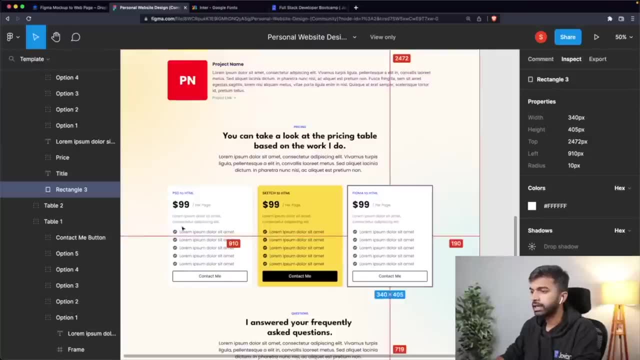 What happens in the pricing section. So it seems like it is 190 pixels out from this side. Okay, And it is about 190 pixels out from this side as well. So one 91, 90,. the total width is 1440.. 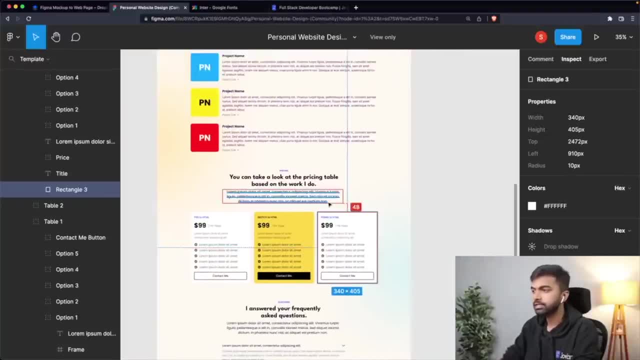 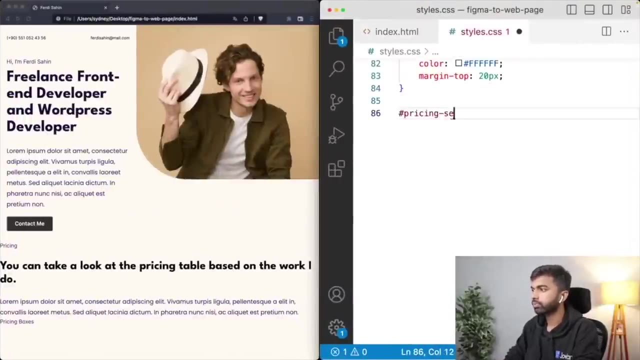 So out of 1440 pixels it is, we are subtracting one 91, four four zero minus one, 90 minus one 90.. That is one zero six zero pixels. So the width of this, or the max width of the pricing section, is one zero six zero max width. 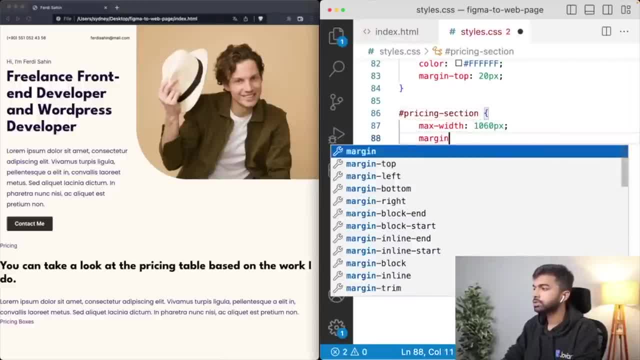 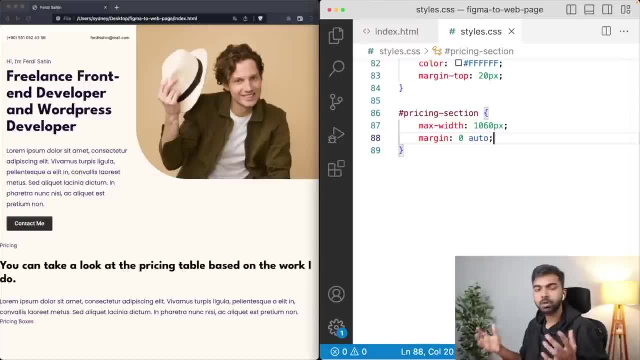 is one zero, six, zero PX. Okay, And I'm also going to set margin to zero and auto margin zero. auto basically says top and bottom margin is zero and left and right margin is auto, which means that you want to compress things into the center. 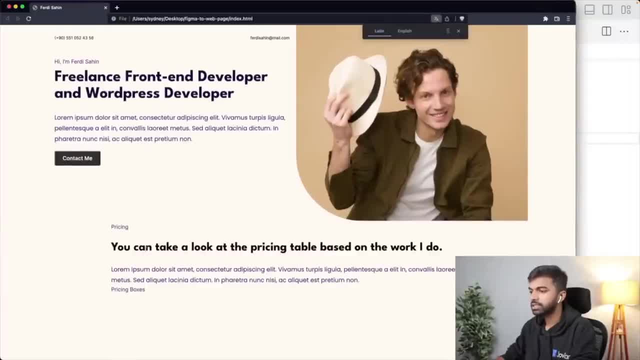 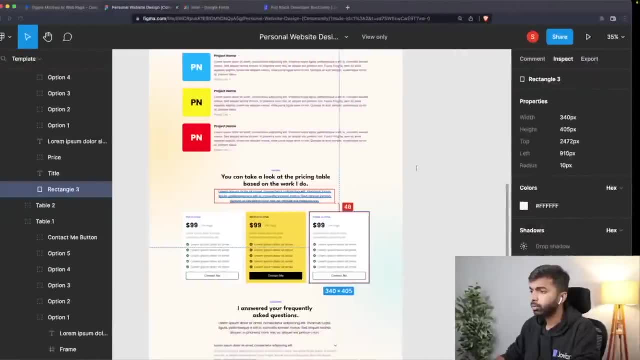 And let's come in here and let's just reload the page and you can now see that it is centered on the page. So it's slightly better than what we had earlier. Okay, Then we have this thing here called pricing over here. It's a very small thing. 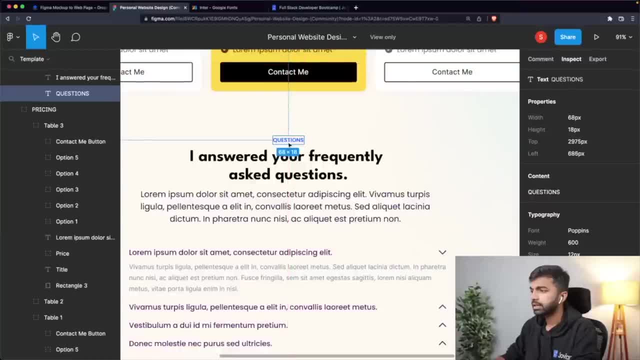 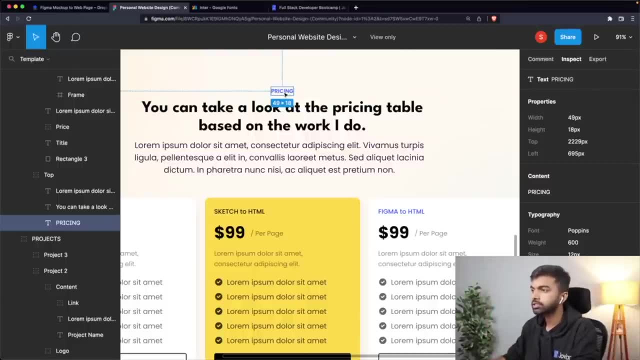 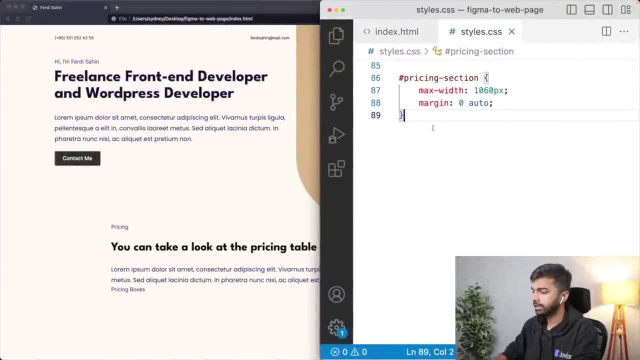 It's in blue color And then we have the same thing later called questions. So let me just call this over title, because it's showing up over the title. So let's just call this over title and let us grab its styles. So I'm going to create a class called over title and let me paste the size here. 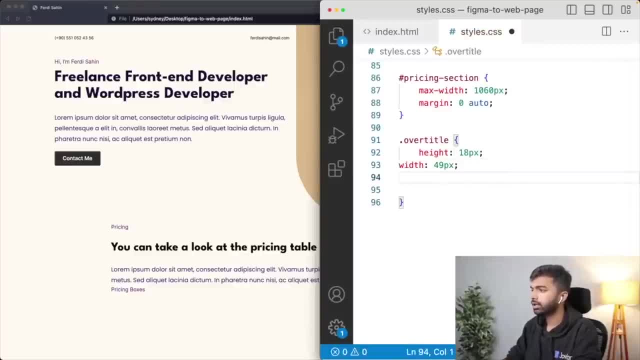 So left and top are not required. We don't need a water radius. So height is 49 pixels, width is no, we don't need a height and width, Okay Okay, We don't need a width either. I think we just need the text styles. 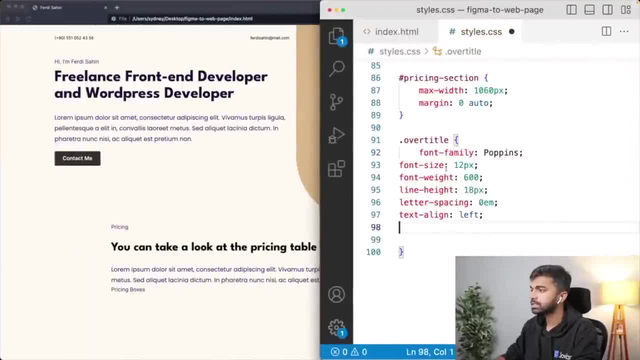 So let's get the text, the typography style. So we are using Poppins and 12 pixels and line height of 18 pixels And we don't need these letter styles. So you have to be careful about which CSS styles you bring in from Figma. 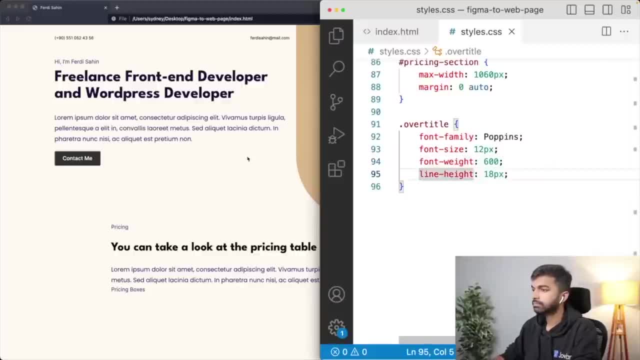 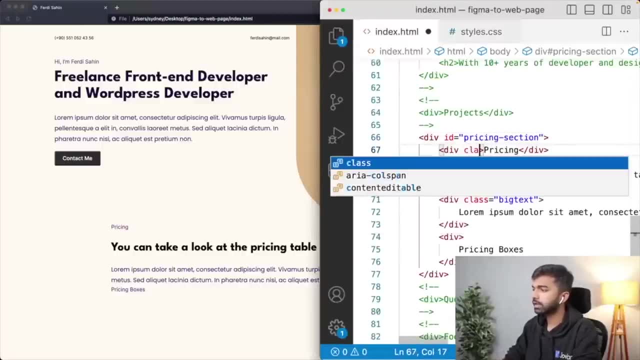 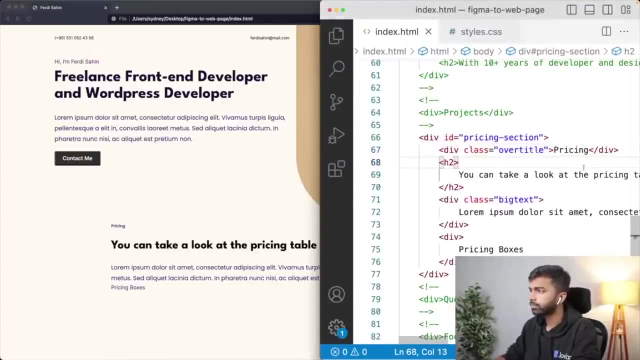 You use it as a reference but don't use it as the ground truth. essentially Okay, And then let's add that over title to this pricing section. So div class equals over title. Okay, And it seems like it's all uppercase. 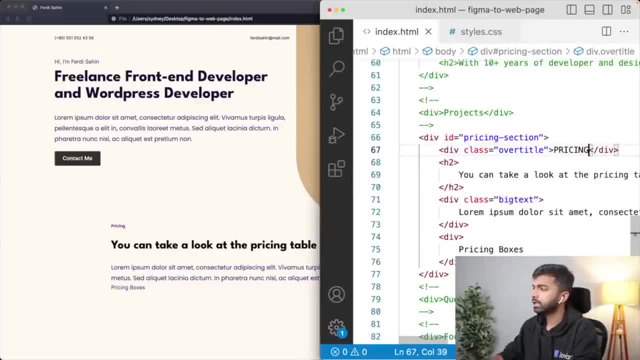 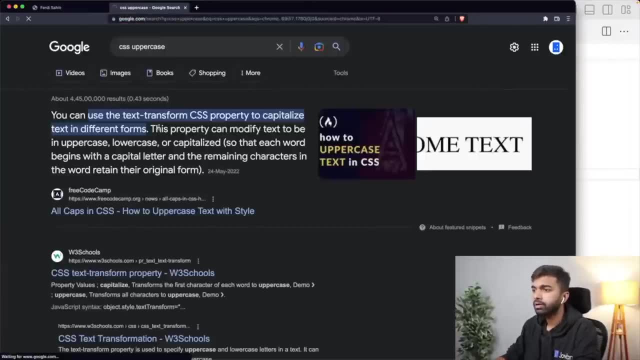 So let me just make it pricing. Actually, we can do it in- I think it's called text decoration. So let me see CSS uppercase. You can use a text transform property. So I'm going to use a text transform uppercase. Okay. 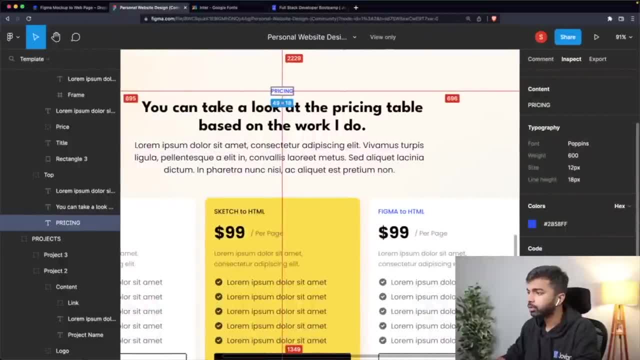 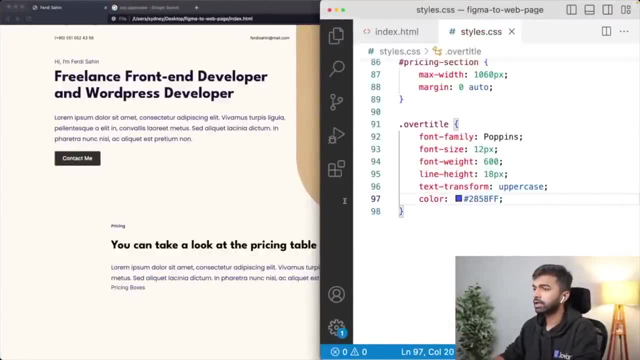 And I'm going to put in the right color as well. It seems to be 2858 FF, Okay, So color is 2858 FF, Okay. So now we have the right price, Now we have the right color. I think we need to add a text align center as well, so that this is centered on the page. 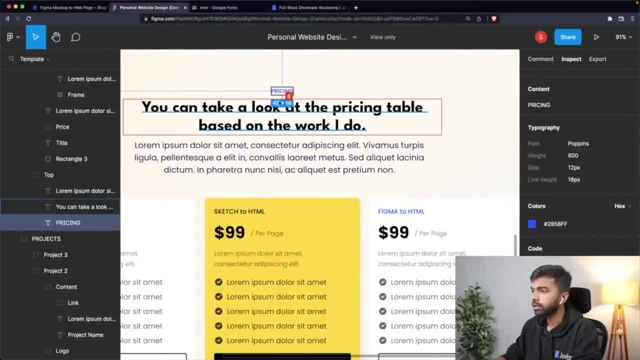 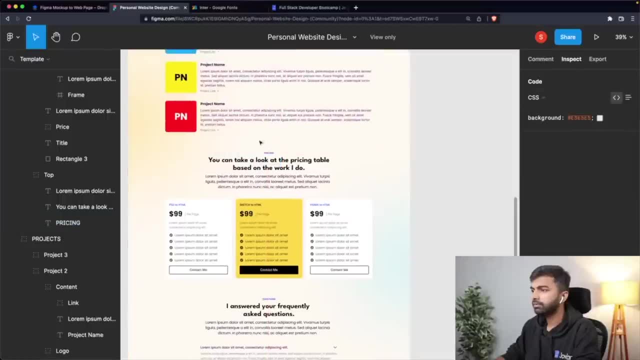 Okay, great. So now this is centered on the page too. Perfect, And finally, I think this is it. But finally, one other thing we have to note here is that there seems to be a significant amount of gap between sections, So I'll have to estimate this. 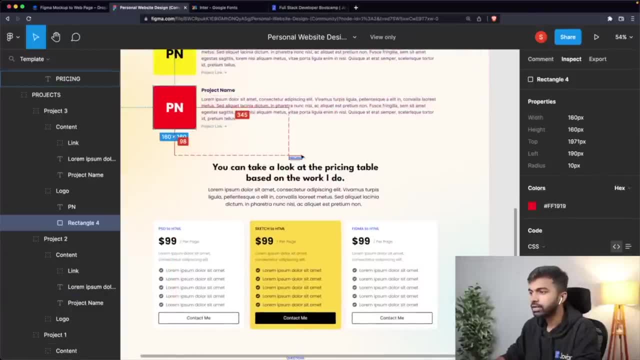 I don't see any direct way of yeah, there it is. Well, 98 pixels seems to be the gap between the pricing section and the. yeah, 98 pixels seems to be the vertical gap. So maybe what we can do is, within the pricing section itself we can add that. 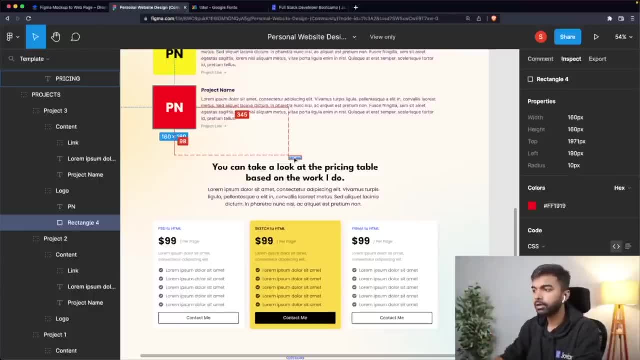 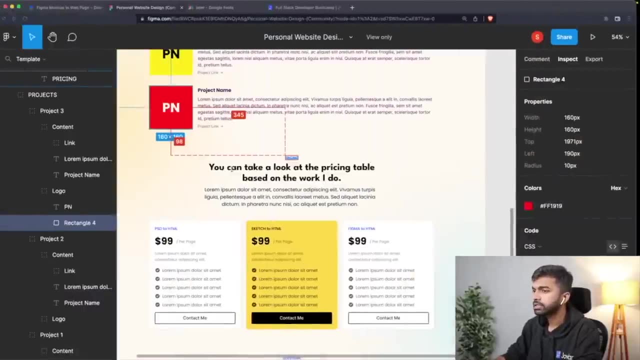 Let's say, each section can have a 40 pixels and a 40 pixels up and down gap, and we can fix the exact things later. So in the pricing section I am just going to say: Well, it's 98, right. 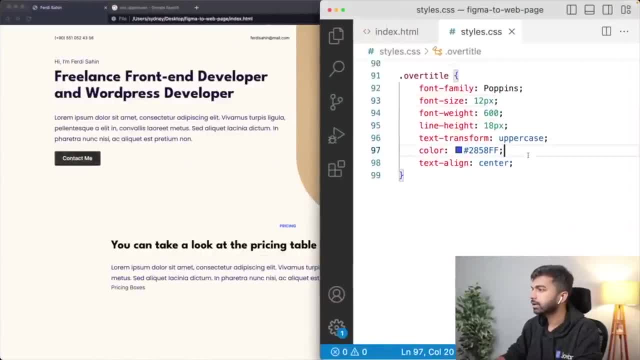 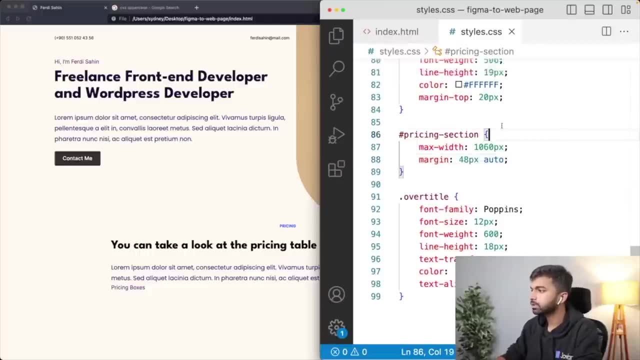 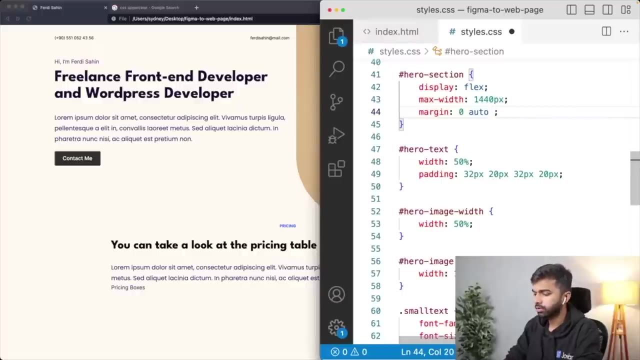 So let me, let me make it 48 pixels. So let's see pricing section. I'm going to say margin top and bottom to be 48 pixels, right, And I'm also going to add a margin bottom for the hero section: zero, auto, 48 pixels auto. 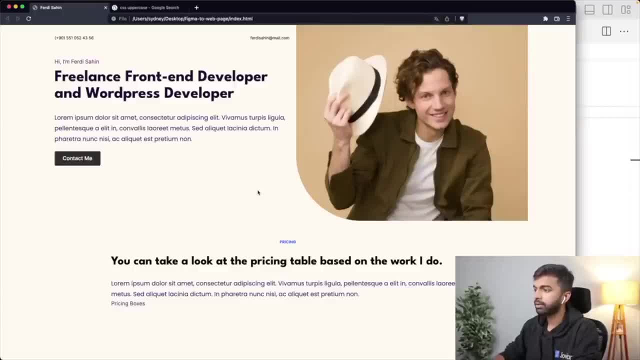 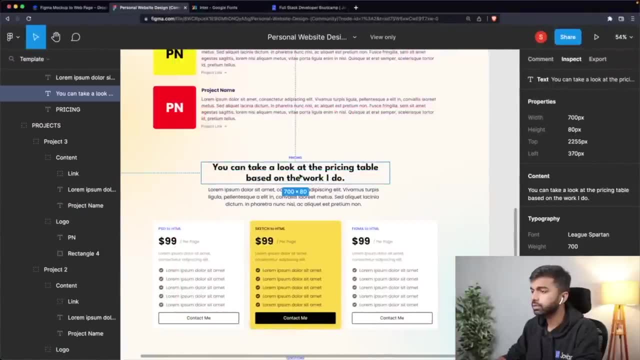 So that between two sections, we have this 98 pixels of gap. All right, So this is looking fine. Now Let's fix this edge too. So we have this edge too. Seems like there is a maximum width, So it's: we are setting a max width of 700 pixels for this. 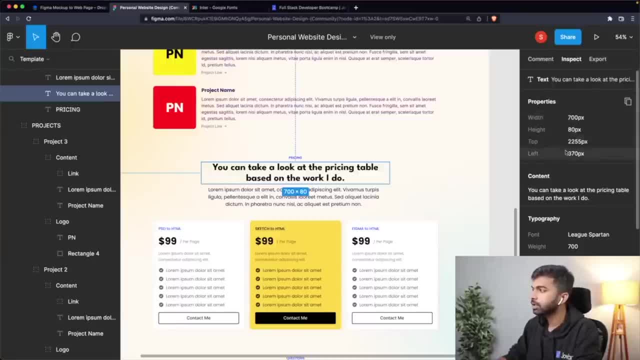 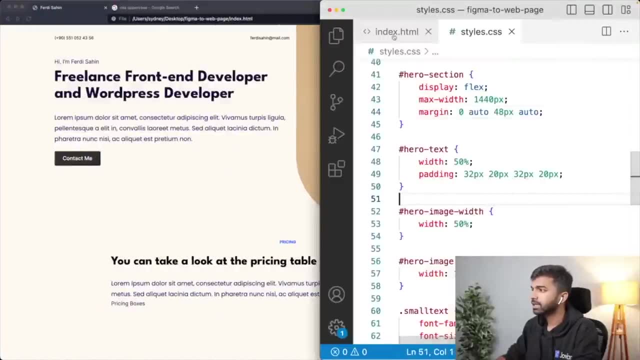 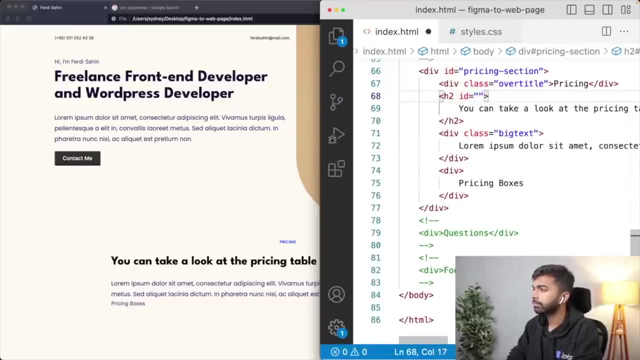 So let's set a max width for 700 pixels for this edge too. Let us also said: maybe text align center. So in this, in this specific case, I am going to say I'm going to give it a hiding, I'm going to give it a ID or give it a class called section heading. 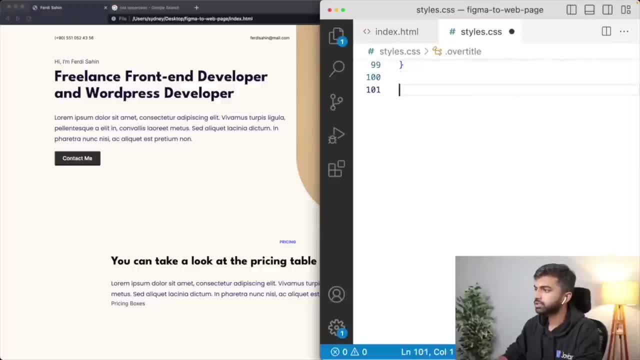 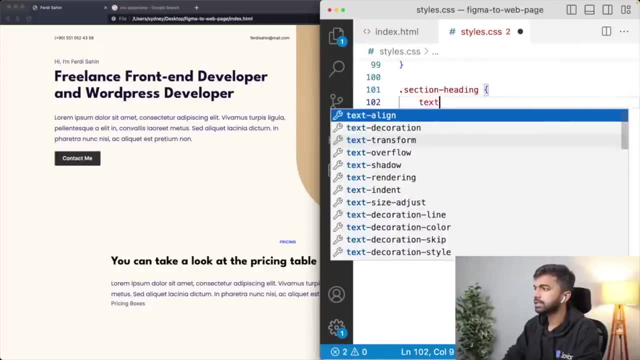 And I'm going to come in because there may be other edge tools which may not be section headings and or dot section heading, And I'm going to say text align center. I'm going to say max width: Let's see 700 pixels. 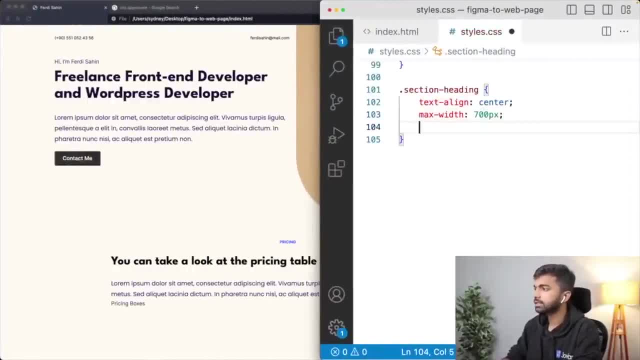 So max width: 700 PX. I'm going to say margin zero auto. so that margin, so that it becomes centered on the page. So if you have something within its parent, horizontally speaking, just give it margin zero auto, And sometimes the zero may be different because you may want to upper and lower margin to 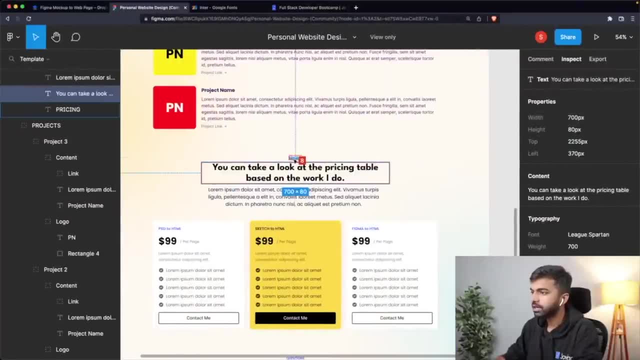 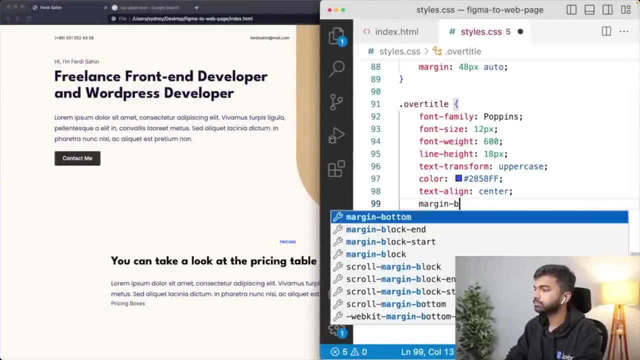 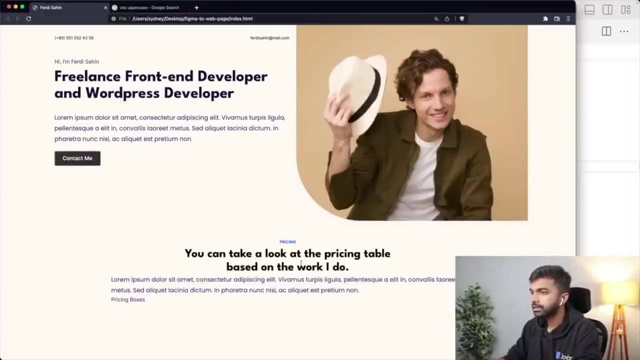 be different, And I think the margin is not exactly zero, but it's eight pixels. So for the over title let me add a margin bottom of eight pixels. Okay, So let's do that. And now you can see suddenly that we now have this pricing section and you can say you: 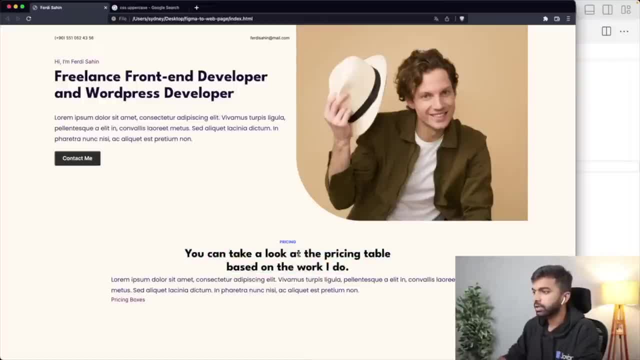 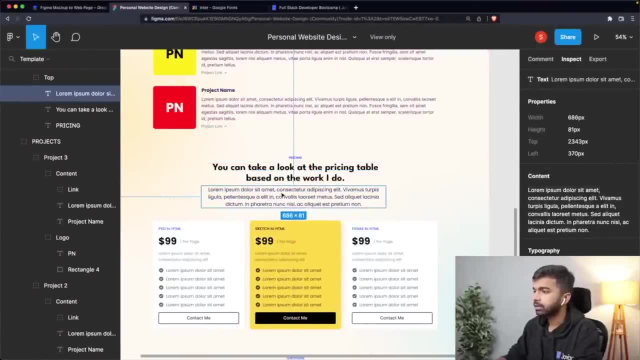 can take a look at the pricing table based on the work I do. So this is good. Now we have the section as well. Let's, let's finally fix this too. So this seems to be the pricing or the section subtitle, essentially. 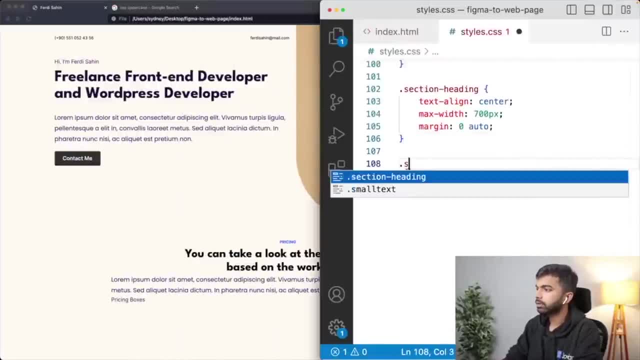 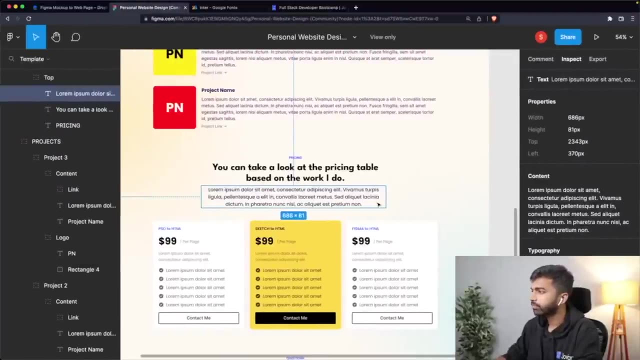 So let's add a class called section subtitle, section sub title, and let us again give it text align center. Let us give it margin zero auto. Let us give it a what is the max width? here, Max width seems to be 686.. 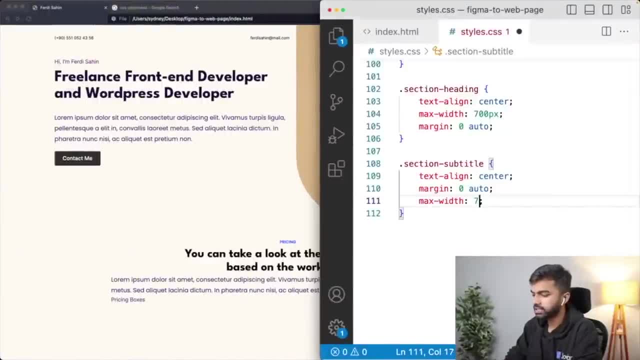 It's about 700.. Let's give it max width of 700 PX And finally, and there seems to be definitely an eight pixel gap. So it's not exactly zero auto, it's eight pixels above And for now let me give zero pixels. 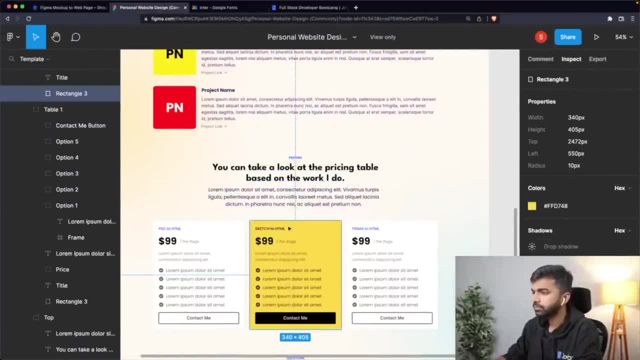 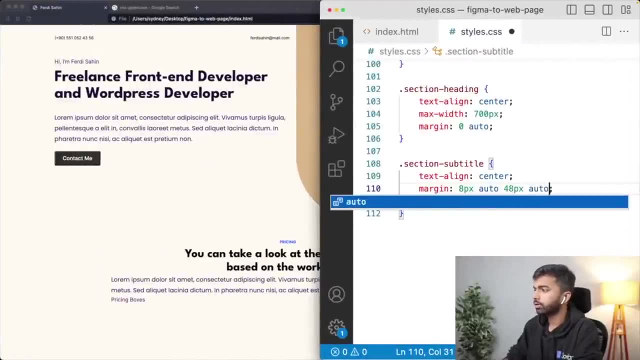 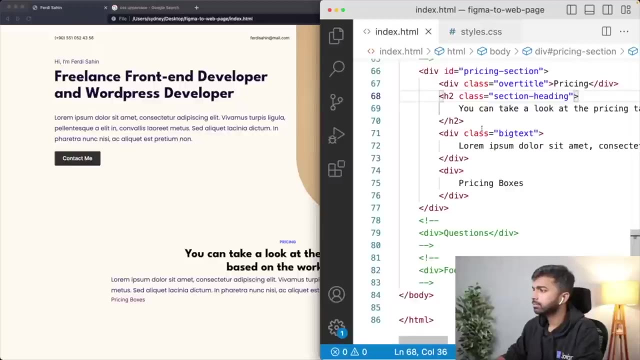 Let's check the bottom distance as well. So let's see 48 pixels below, right, So eight pixels above, 48 pixels below, and then auto, All right. So with that, and text align center as well. oh, we need to add the section subtitle. 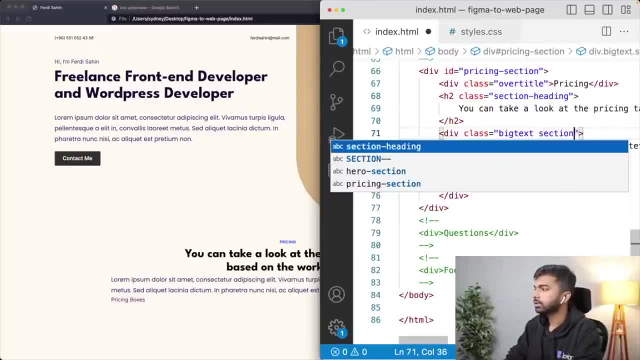 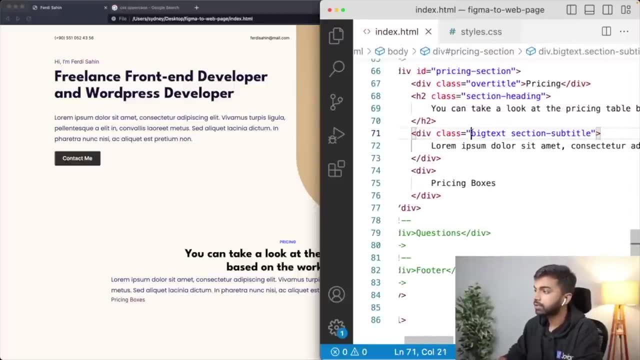 So we can add a second class here. section subtitle. So this is how you add multiple classes: You can add not just one class, but you can add multiple classes to a div. So we have big text and we have section subtitle. 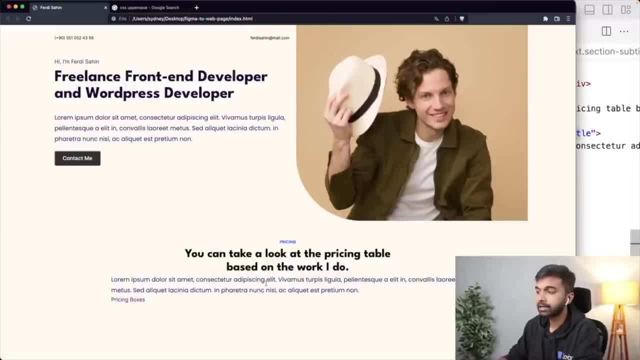 So big text is going to ensure that it gets this font size and it gets this color, and section subtitle is going to ensure that it is centered on the page, as we might expect, Right. So now you, now you can see, now we have this pricing section. 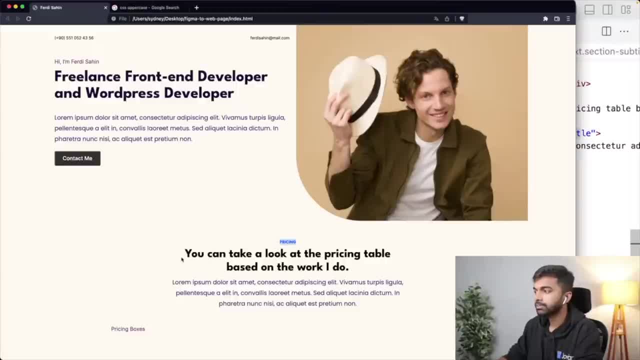 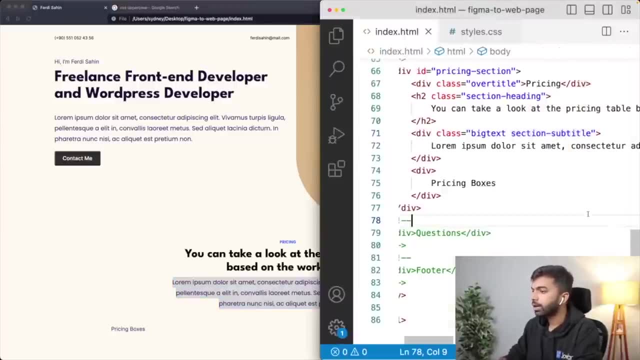 And in this pricing section we have the title. in this pricing section, We have this and we have this content as well. Okay, great, So things are looking good. Let's finally go ahead and maybe try to also add the pricing boxes. 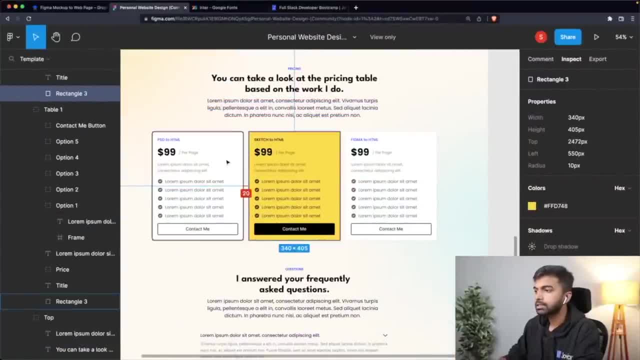 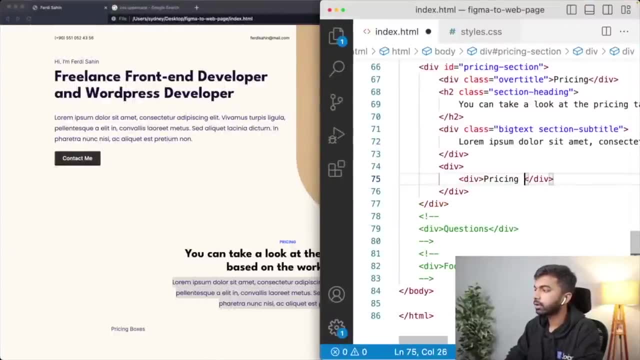 I think if we can add one box, we should be able to add all the boxes. So let's come back here and let's: there are three pricing boxes, So let's create three divs. So let's call it pricing box one and div box two and div box three. 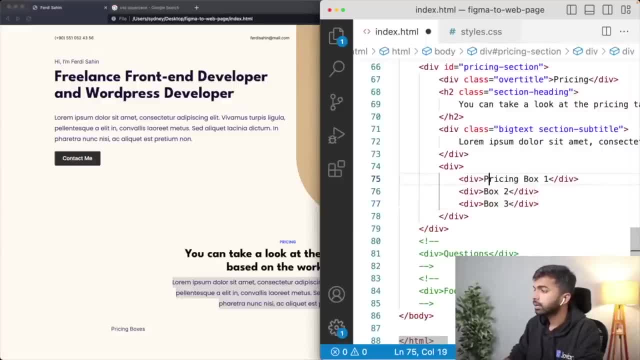 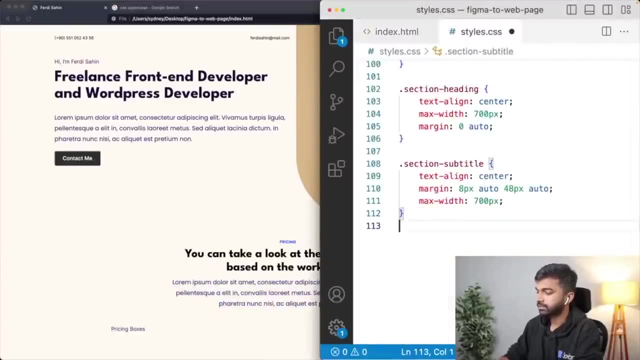 Okay, And now into this div, I let me give this a ID pricing boxes. Okay, I have given it to the. I've given it an ID pricing boxes. So I'm going to come back into my styles file and for the pricing boxes div, I'm going to 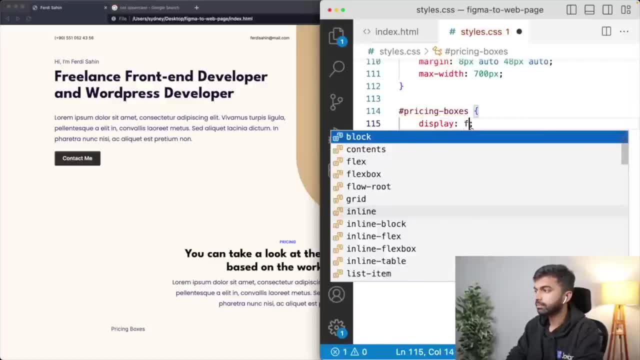 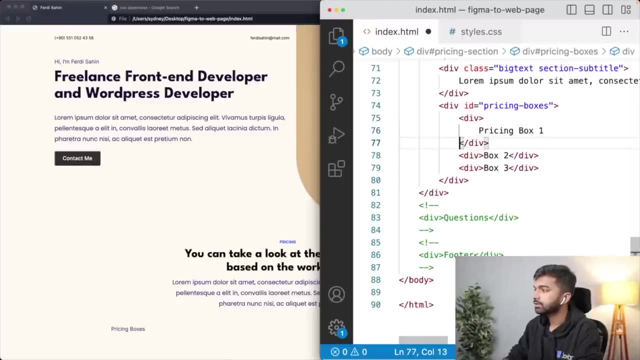 say: display flex. Okay, We want to flex. We want the? Okay, We want the children of this div to be horizontal. So display flex. And let me give all of these a class pricing box so that I can set each of their widths. 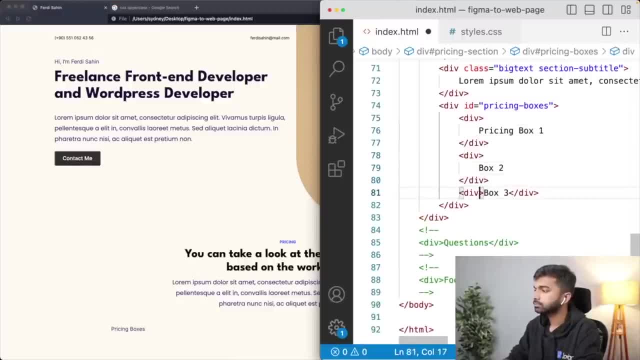 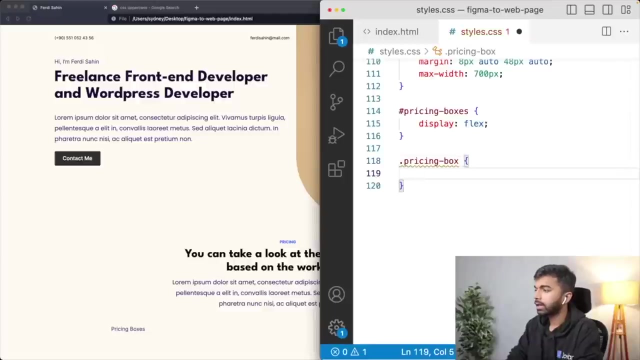 to 33%. Let's see class equals pricing box And let's add that to all of them. You can also use advanced flex box properties to do this, But for now I'm just going to use something very simple and I'm going to set for width. 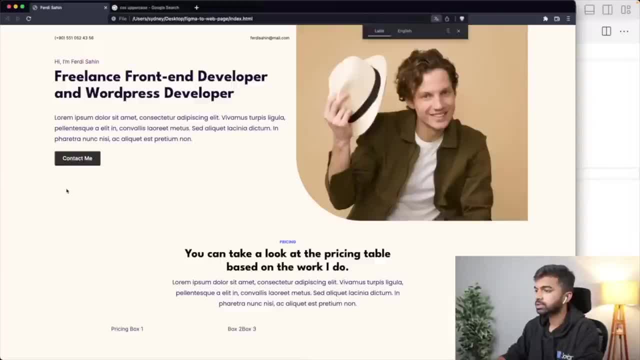 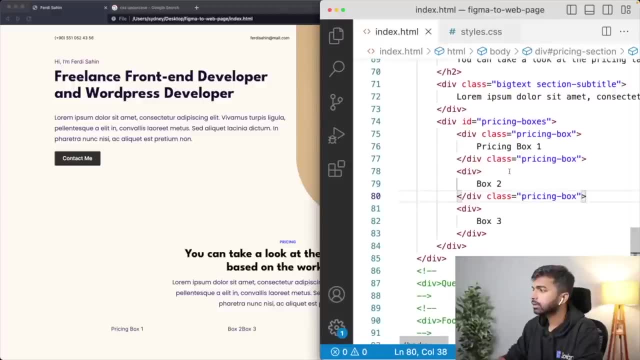 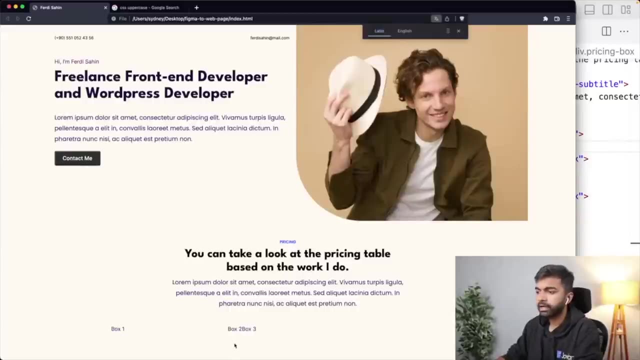 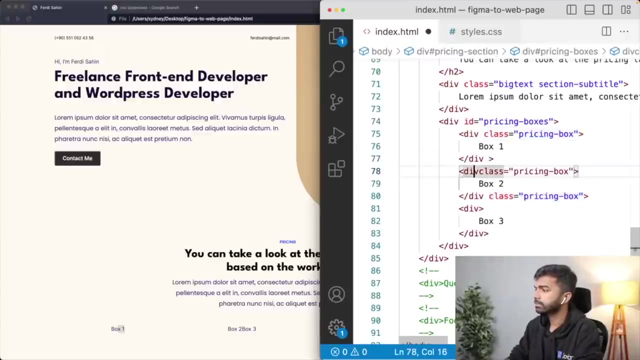 of 33% for a pricing box. Okay, And yeah. So now you can see that we have at the very bottom we have box one, box two and box three. Okay, I forgot to add the class here. I added it in the wrong place. 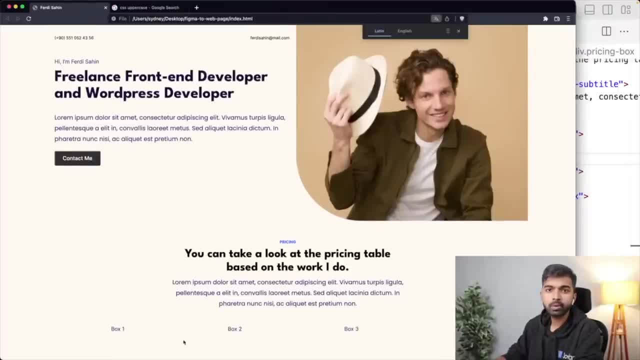 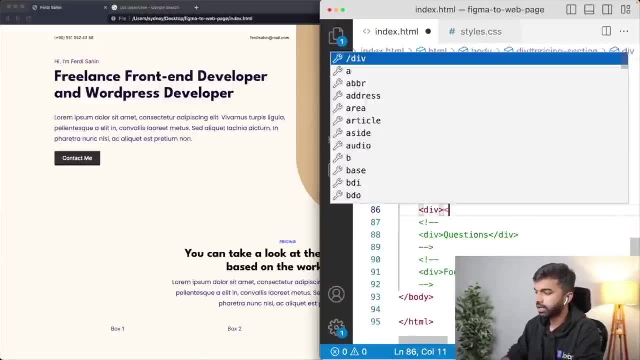 Yeah, So now we have box one, box two, box three, at the bottom of the page. I'm just going to add a small div with a large height at the end, just so that we can bring up some of these pricing boxes. 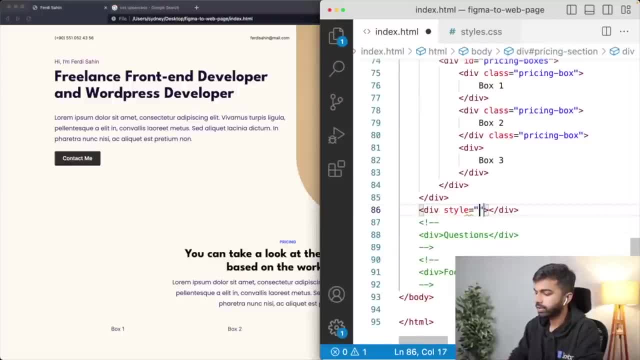 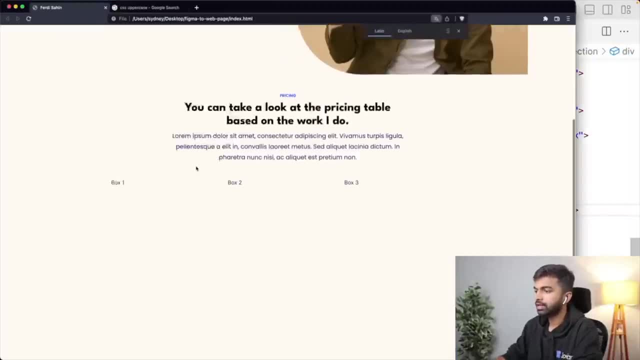 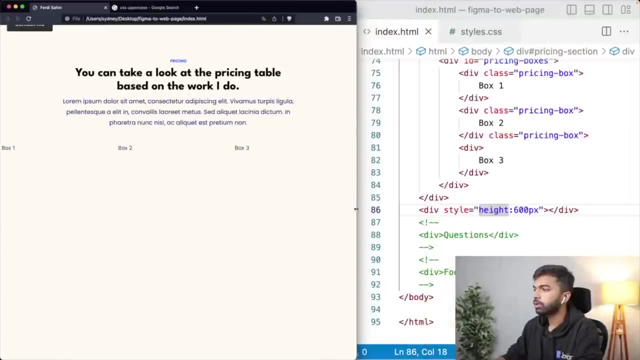 So I'm just going to give it style: equals height: 600 PX. This is just to add another div at the bottom so that I can scroll this up a little bit while developing. Okay, And then we want to create these boxes. So what do we want to do in these boxes? 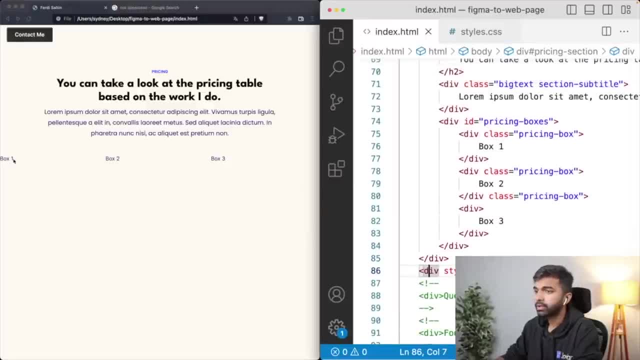 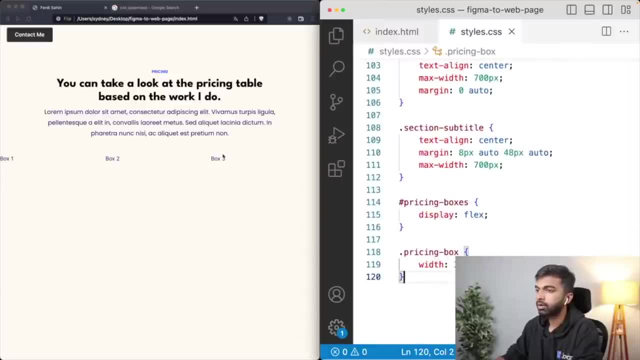 Let's see one by one what we are going to do in these boxes. By the way, you can see here- pricing boxes- We may also need to add a little bit of a padding So that it's not sticking to the corner, but we'll figure it out. 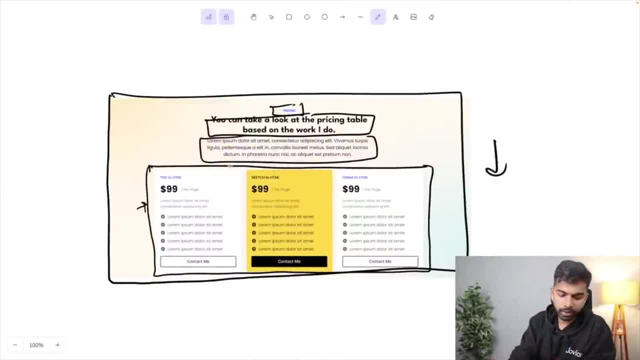 Okay. So coming back here to the design, what we've already done is we figured out that we need a vertical or we need a horizontal layout here. That's why we use display flex. And then we have these three boxes. Yeah, Each box seems to have equal. yeah, each box seems to have equal width. 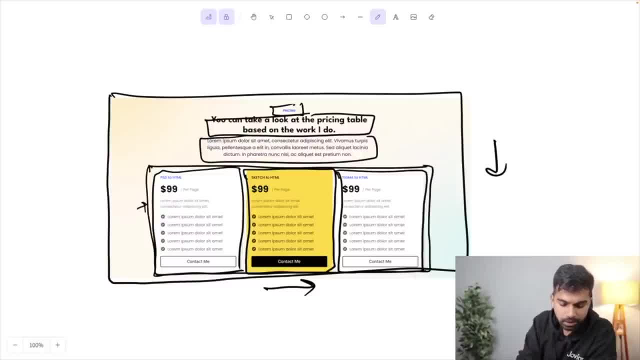 We've done that with 33% width. Now, in a particular box, the layout seems to be vertical. Okay, So we have a bunch of these and in a vertical layout, if I start drawing boxes, we have one, two, three, four and five boxes. 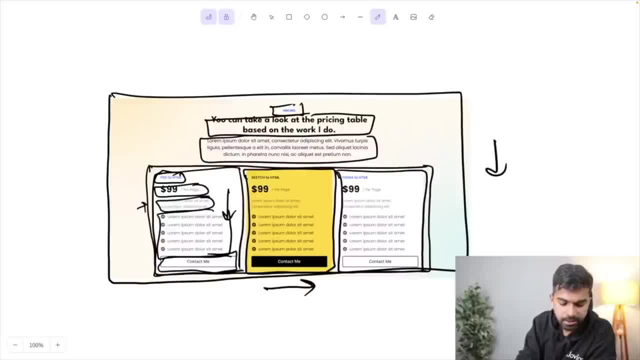 Okay, So I'm going to connect PST to HTML, which is a service. One is the price, Then one is a description, One is the. these are, let's say, benefits and a contact button, right? So let's do that and let's add, let's start adding all of these. 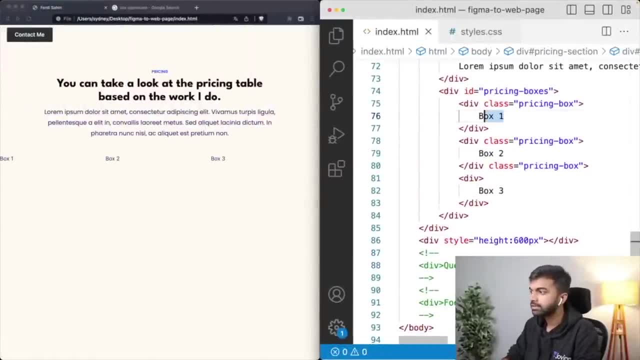 So in the pricing box one, I'm just going to do one box and let's see if we can maybe just copy paste and use similar styles wherever possible. So I'm going to create a div. Okay, So I'm going to give it the class service. 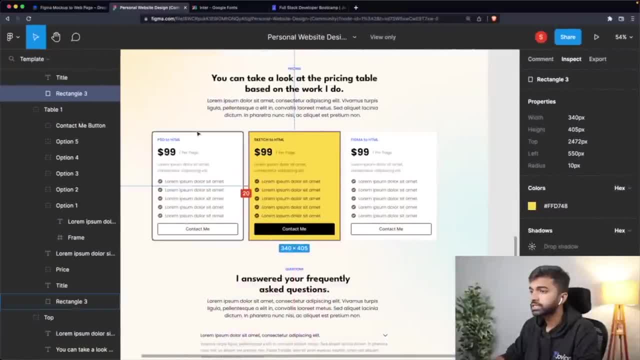 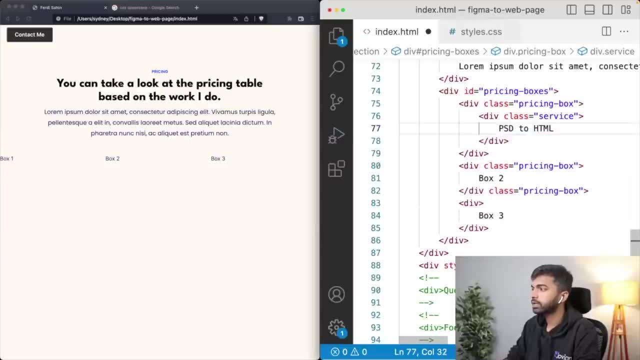 And what is the service here? So the service here is PSD to HTML. So let's just say PSD or PSD to HTML. So that is a service that is offered in the first pricing box. Then I'm going to have another div here. 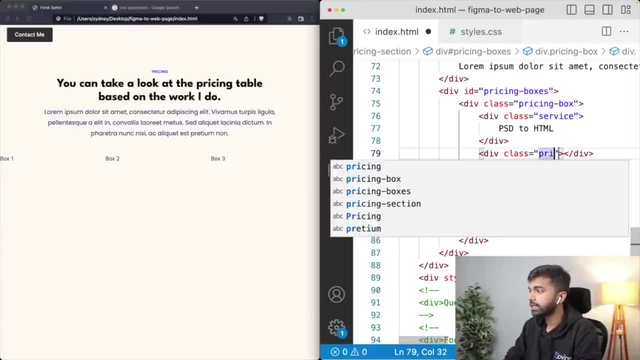 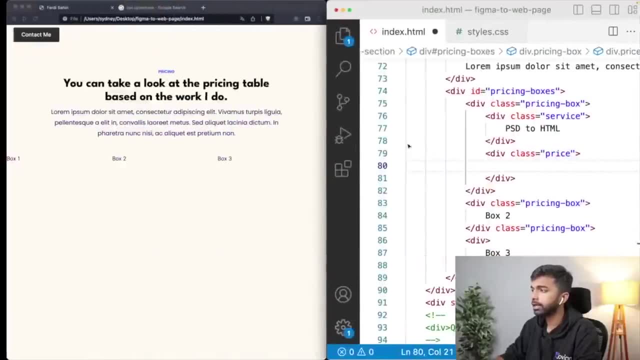 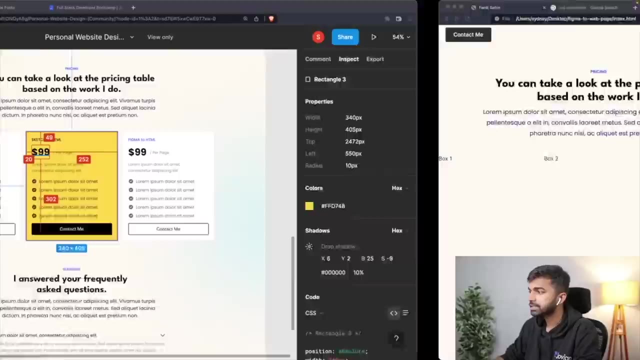 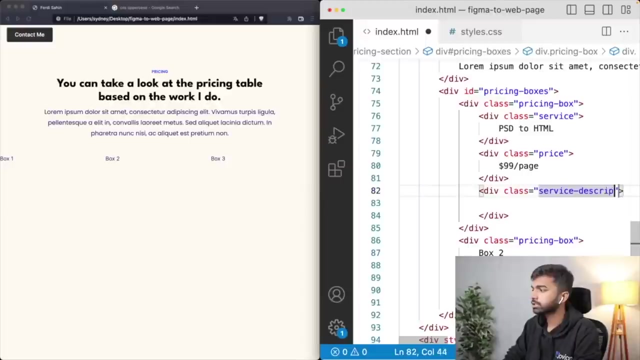 I'm going to give it the class price. So the price For the first service is $99, $99 per page will fix the styling later. Then let's add the description, So let's say class service description. So it's good to be a little specific with class names because description is a very 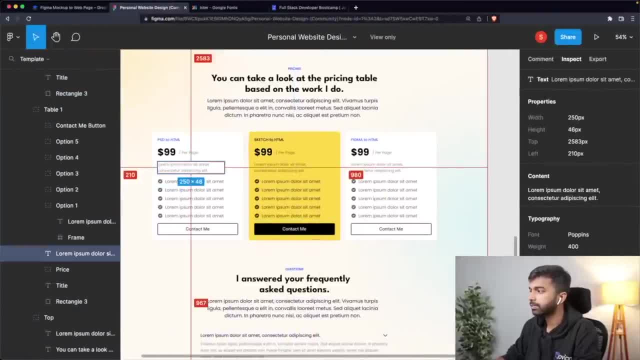 generic, very generic class name that may apply to a lot of things. So let's copy that content, Let's put that in content in here, So this description. then let's go in and let let's call these service benefits. So this is a list. 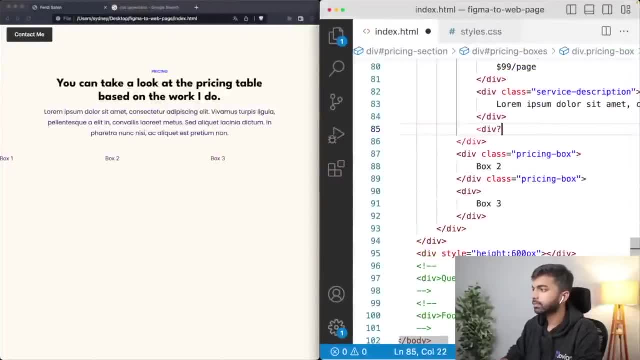 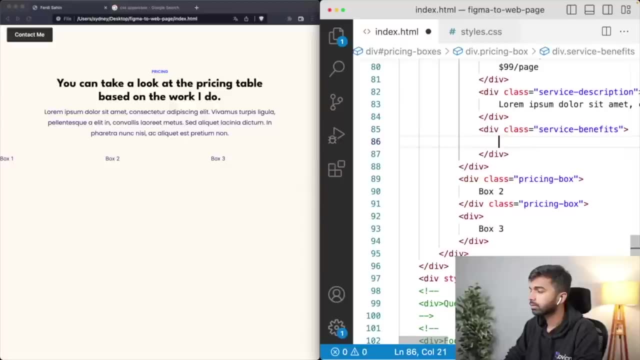 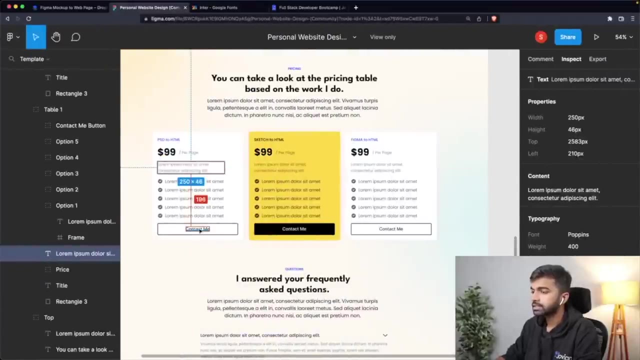 So I'm just going to create a single div for this. Let's give it the class service benefits, Okay, and let's just put service benefits here. And finally, there is this service contact button, right? So let's put in a button here. 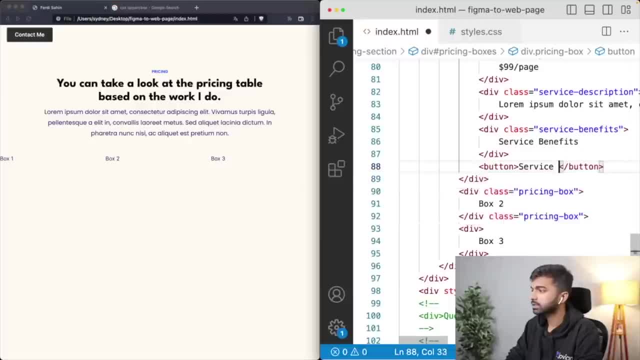 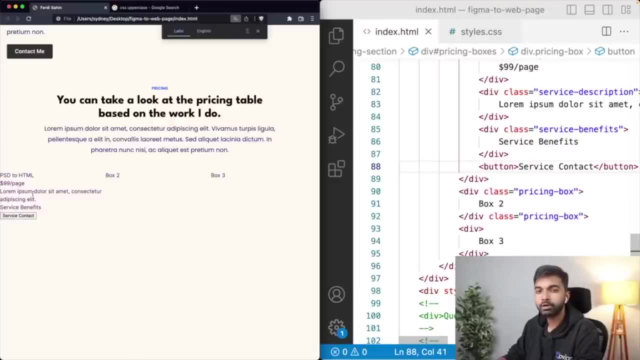 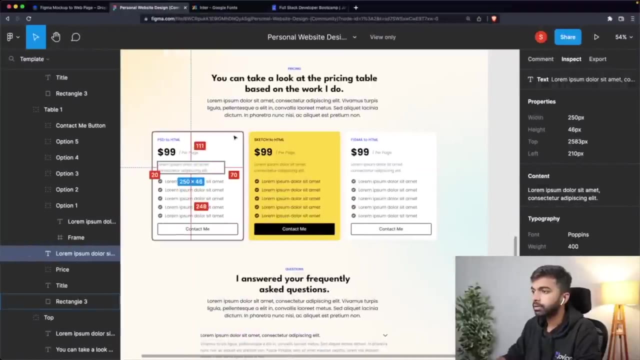 And let's just say service contact. All right, so now we have some content here, And of course this is not looking exactly how we want. But now for the first box. we have some content in place. Now let's start actually laying out the box. 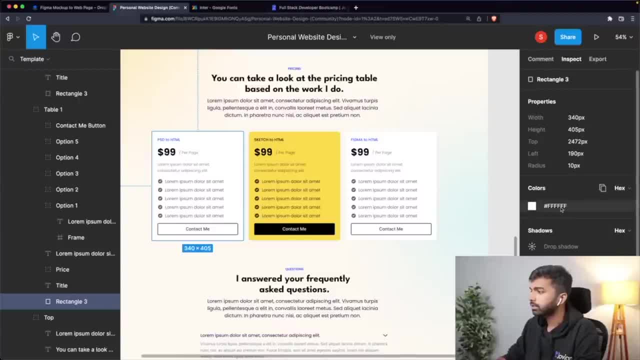 So this box by itself seems to be a, seems to have a white background. So let's do that. Let's, let's end. the different boxes have different backgrounds, So maybe background is not something that we want to set, Let's set it. 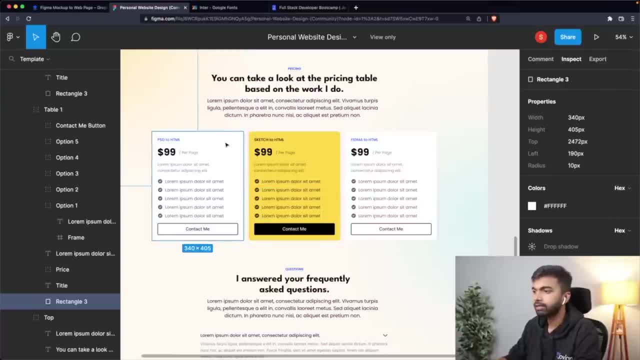 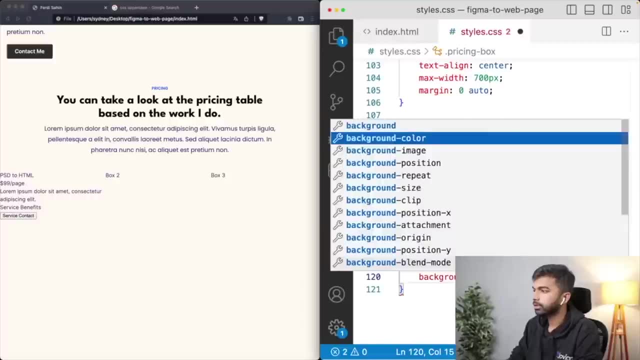 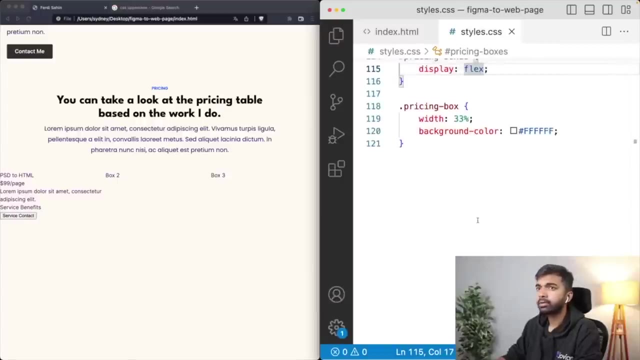 That's okay. Let's set on pricing box itself. Let's set the background and, if required, later we can change it. So pricing box should have the background or background color white. I've added the background color of white for pricing box. 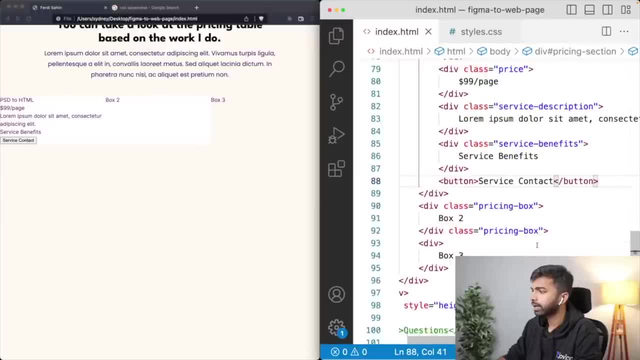 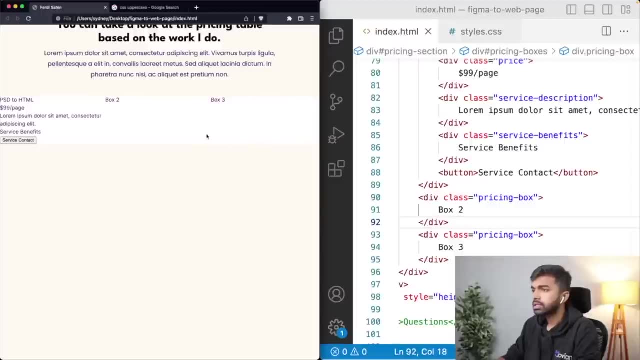 So now you can see that each pricing box has the background color white. Oh, the third one is not given the right. Yeah, So these pricing boxes have the background white, but they seem to be touching. We don't want them to touch. 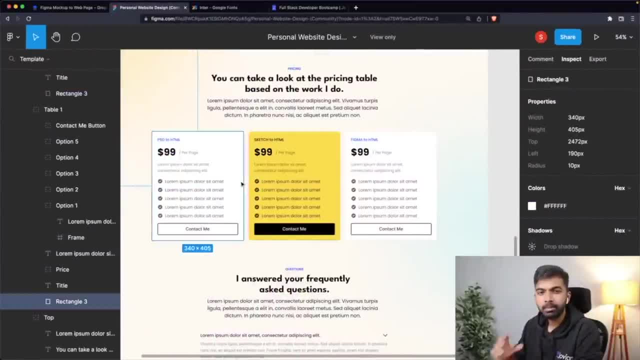 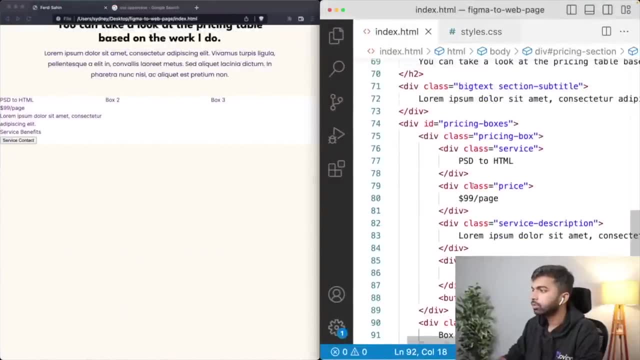 We actually want a 20 pixel gap between them, or maybe a 10 pixel gap around the box. So here's a quick trick that I'm going to use. I'm going to create a new div called pricing card. So div class equals pricing card. 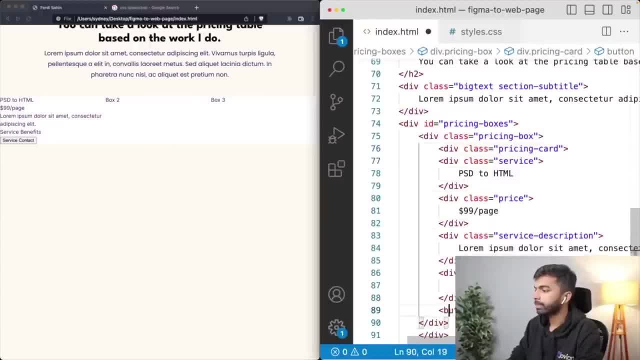 And I'm going to put everything inside this card. Okay, So I'm going to keep the outer div just to determine the width of each width of each of the boxes, And I'm going to actually use a pricing card which is going to have the margin which is: 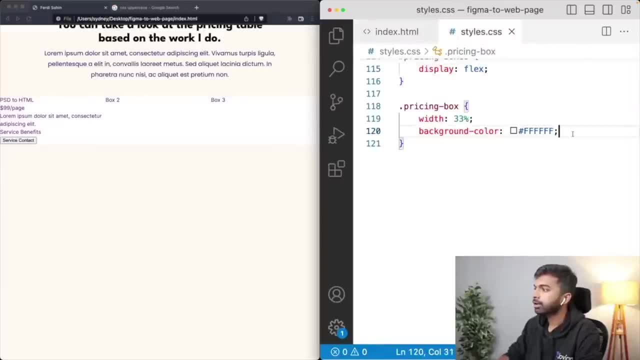 going to have the shadow and all of that, Okay. So instead of adding the background color on pricing box, let me add it on pricing card. and background color is okay, FF. And let me add a margin of zero pixels at top and bottom. 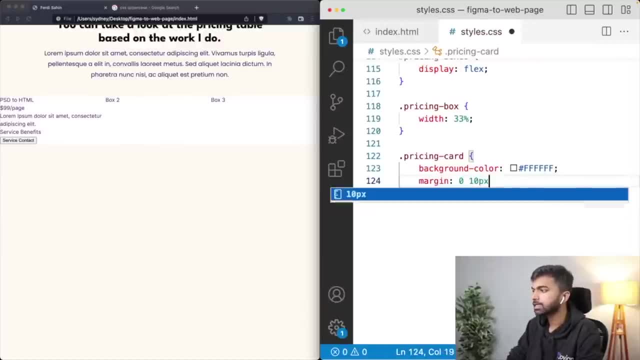 We don't need it, We don't need that. But left and right, let's get a 10 P X margin. Okay. So now the benefit that you get is that, inside the pricing box, which determines simply the bit, 30%, 30%, 33% or let's actually just do that 33.33%, just to be very accurate. 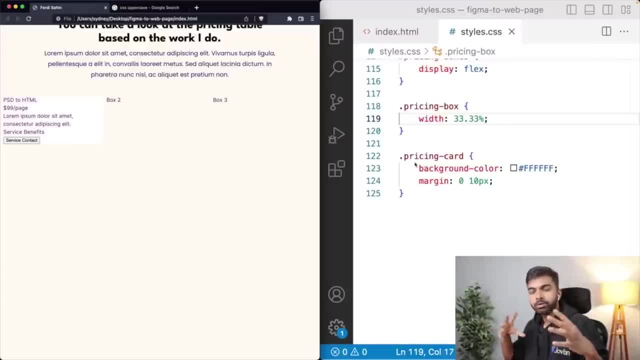 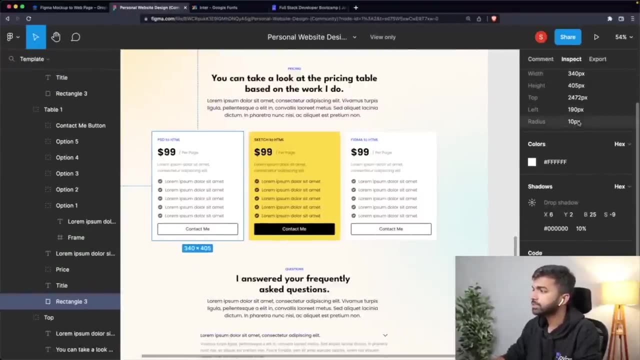 And then we have this card. This card is going to be inside the box that is going to have some margin around it. It is also going to be habits, rounded borders and all. So the radius, okay, The border radius Seems to be about 10 pixels. 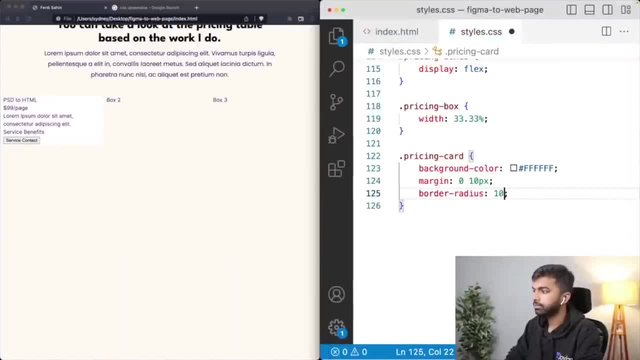 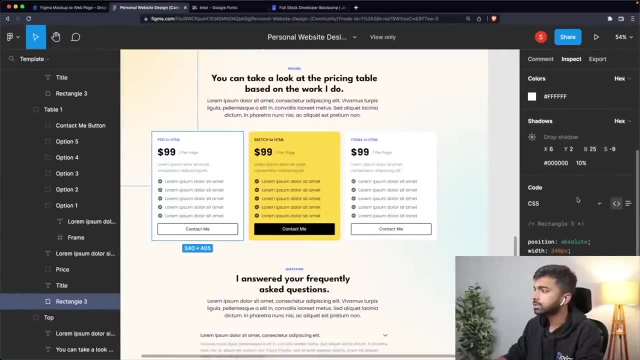 So let's add a border radius. border radius: 10 P X. Okay, Now border radius has been added, Then it seems to also have a shadow, So there seems to be this drop shadow. I think we can just copy this drop shadow setting and paste it in here. 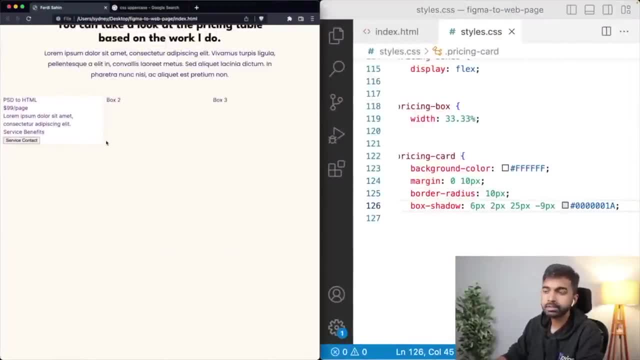 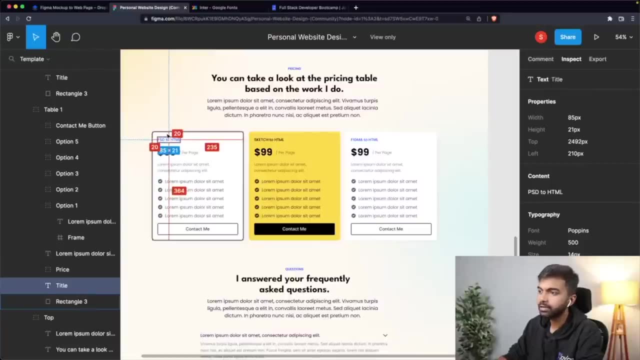 So it seems to have a box shadow. So now you can see here that it has gotten a shadow as well. So that's good, Now we have a shadow. then inside it seems to have about 20 pixels of padding. inside. You can see that all the content is padded by about 20 pixels. 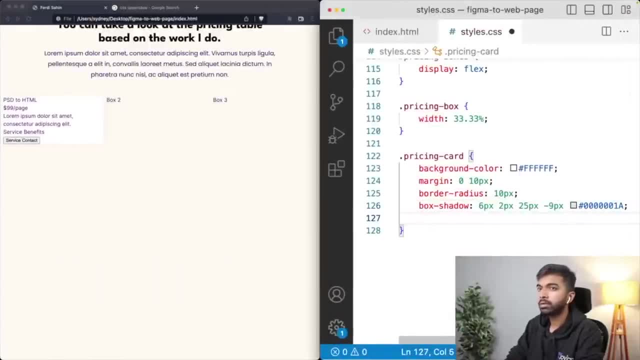 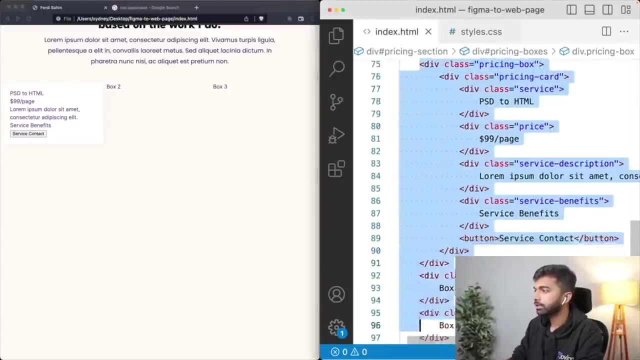 So let's add a padding all around of 20 pixels, Yep. So now we have a nice padding as well, And what you can do just for now is I can just copy over the same content into the other boxes as well And we let it the content later. but the benefit of that will be we'll be able to. 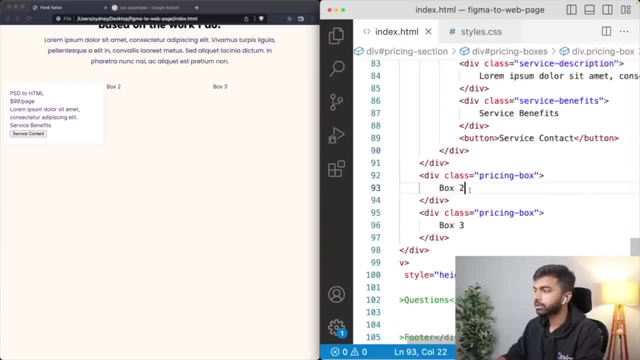 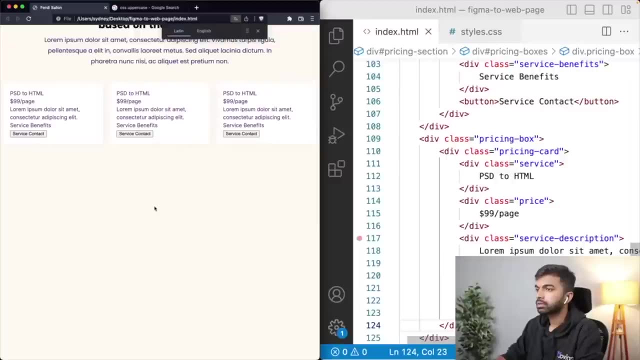 see that How we, as we modify one particular class. Okay, So that's going to apply to all of the different boxes at once. Okay, Yeah, So now we have. okay, now we have these pricing boxes, and these pricing boxes seem to be looking. 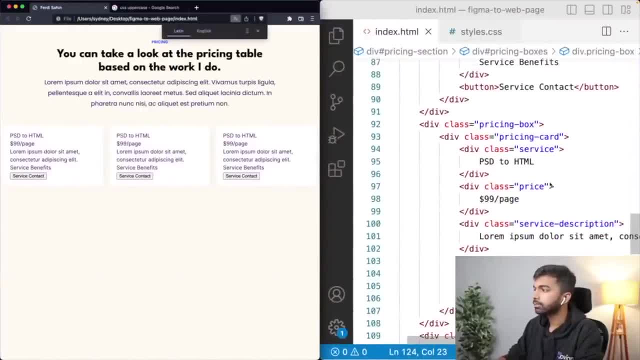 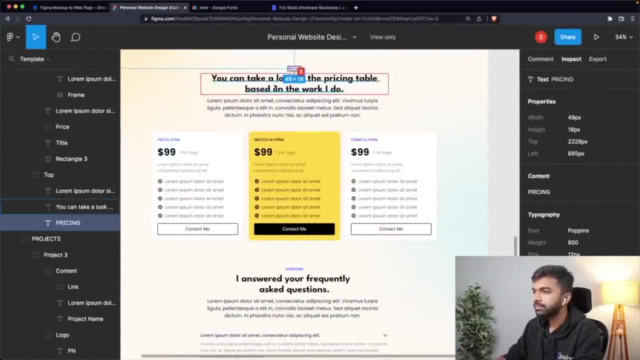 at least on the outside, as we expect them. And now we can start modifying the service, the service, the class for the services. Let's see. So this is probably the same class. No, it's a slightly different class, but it seems like it has a. let's see. it has this: 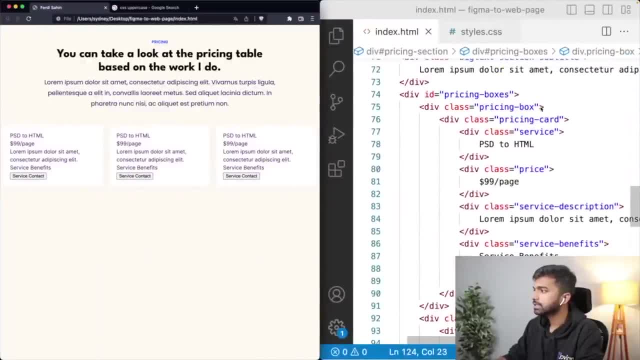 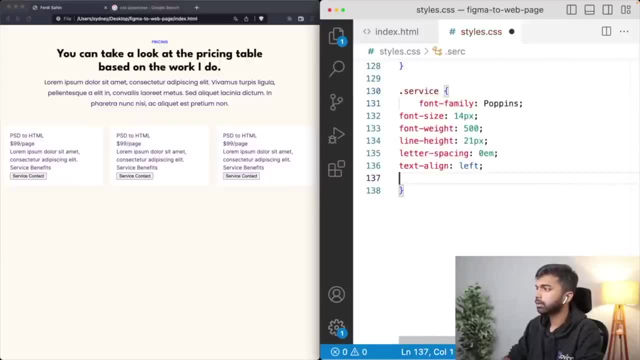 font pop-ins. So price service is the class. So for the class service I'm going to add the font color or the font settings. font: family pop-ins. Okay, Font size: 14. line height is 21.. Get rid of these two. 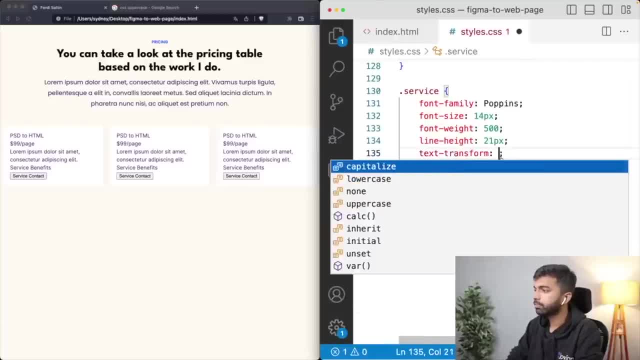 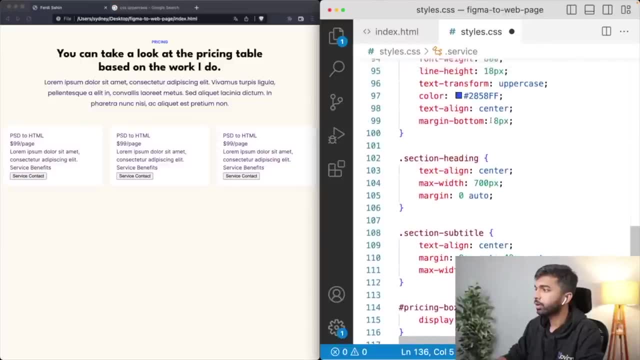 Let's add, maybe, the color as well. Let's add the text: transform upper case and let's add the color. I think it's the same color as a pricing section over title, which is this: Okay, So let's add the color here. 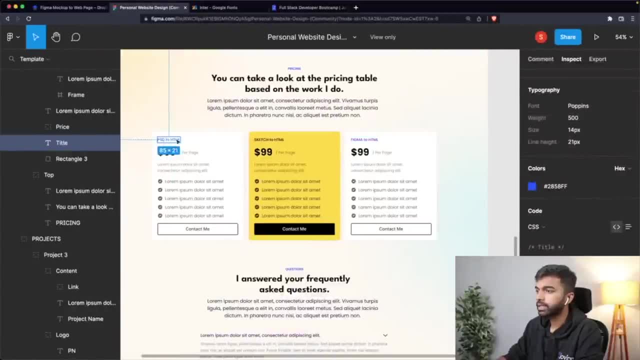 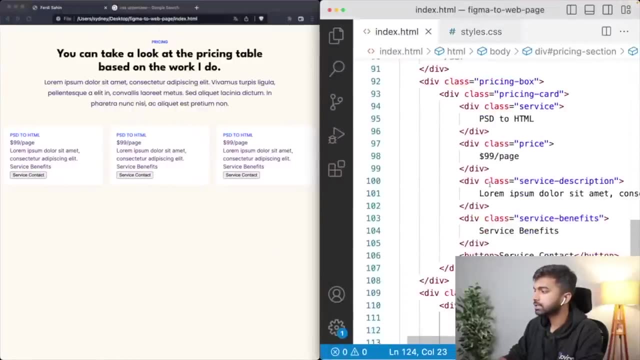 Okay, So now the services are looking good: PSD to HTML, Sketch to HTML, Figma to HTML. Okay, Well, I'm just going to edit those as well. So I'm just going to say: for box two, I'm going to say Sketch to HTML. 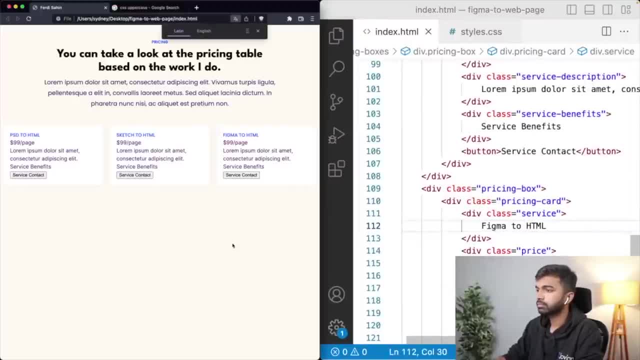 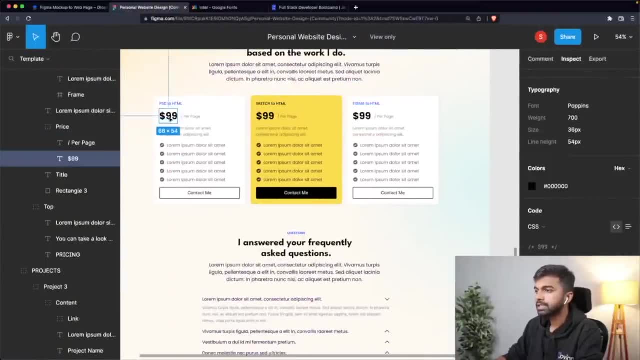 And here I'm going to say Figma to HTML. Yeah, So PSD to HTML, Sketch to HTML, Figma to HTML: 19.5.. 99 per page. Let's get the styles of 99.. So the style here is pop-ins and line height is 54,, size is 36,, weight: 700.. 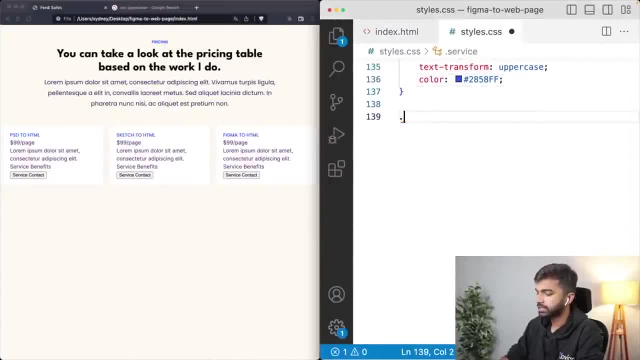 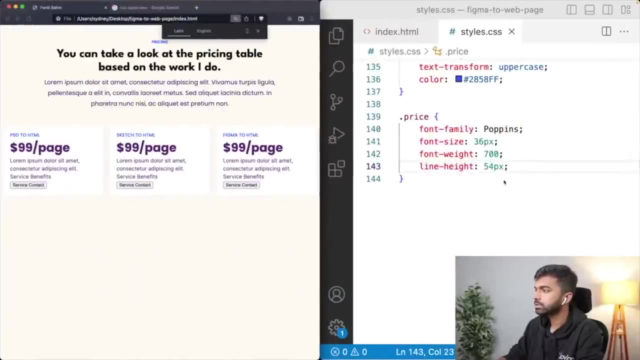 So this is the price. So let's add the styles for price, dot price. Okay, All of this looks good: Font size, line height, all of this looks fine And the color seems to be just black. So I'm going to say color. 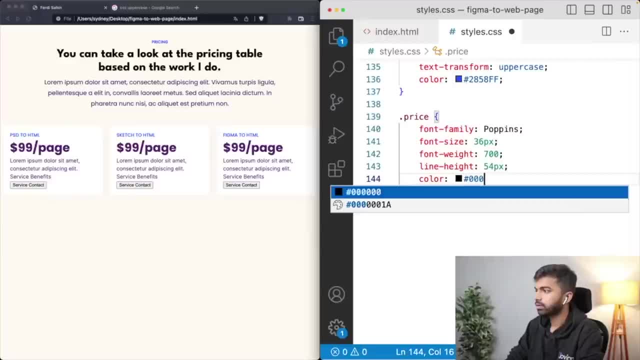 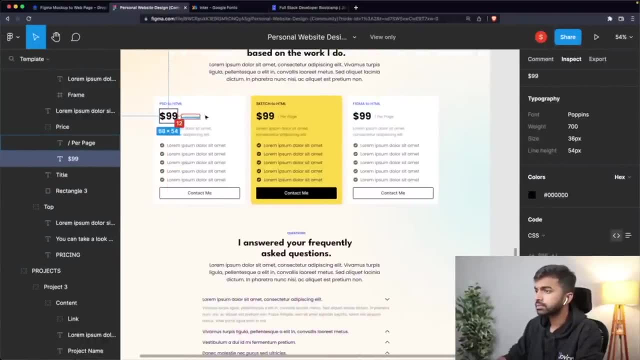 0, 0, 0, 0, 0, 0.. Okay, The color is fine too. Then, okay, This slash per page. So this information. I think this is something that we can put under the span probably. 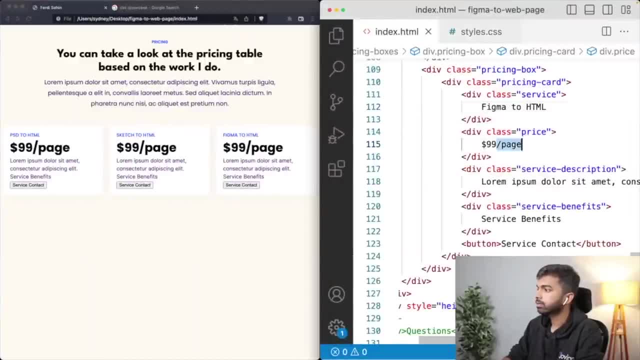 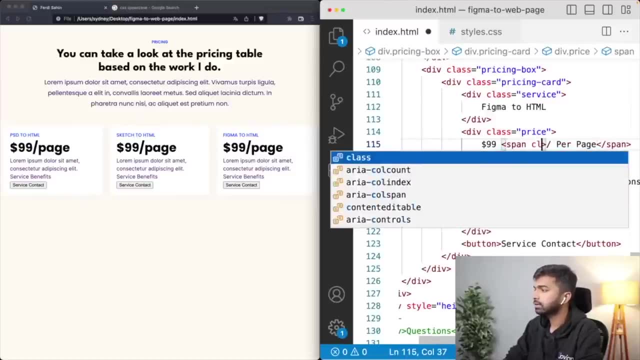 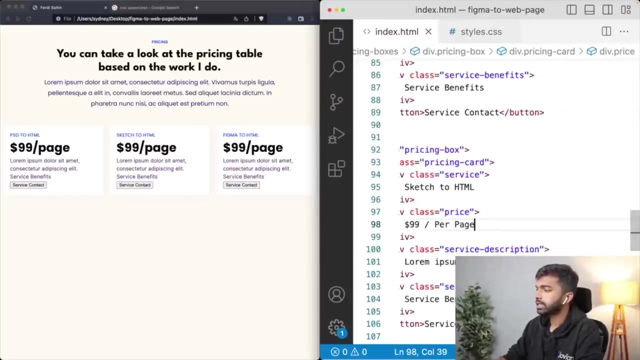 So I'm just going to put a span around this Span and I'm just going to give this span A click. Okay, Class of price per okay. So let me just copy that and paste it in the other ones as well. 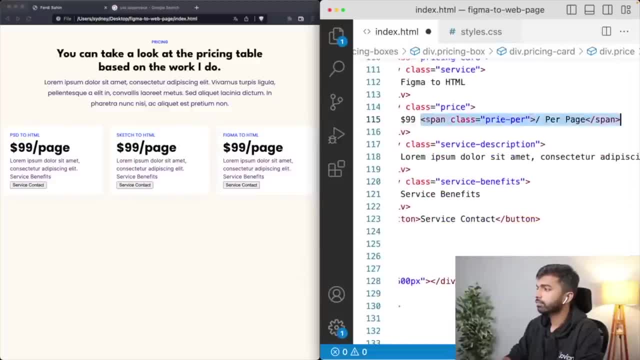 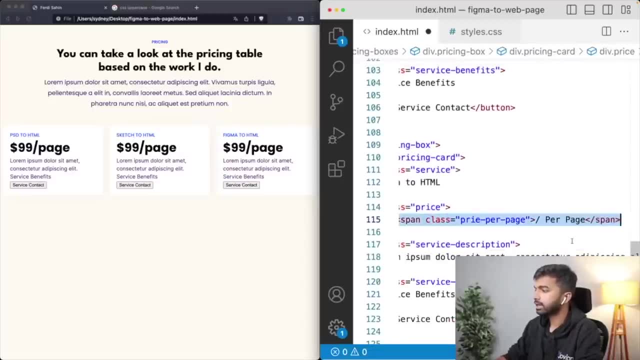 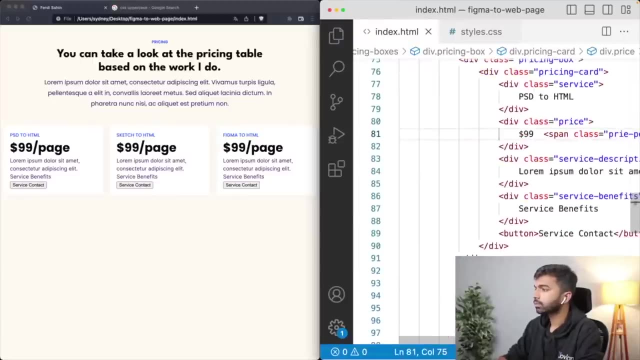 Price. oops, Let's copy this whole span or price per page. Let's give it a class of price per page. Let's copy the entire span and let us put that span in each one. Okay, Price Per page. Price per page. 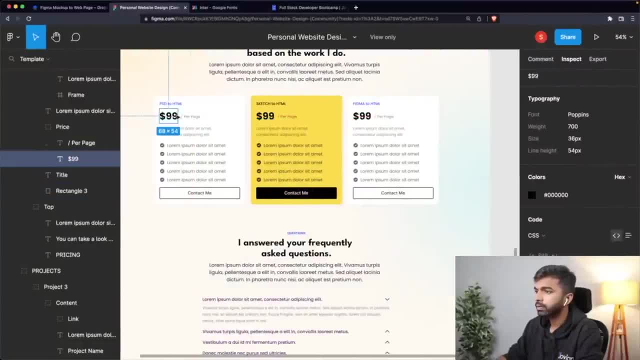 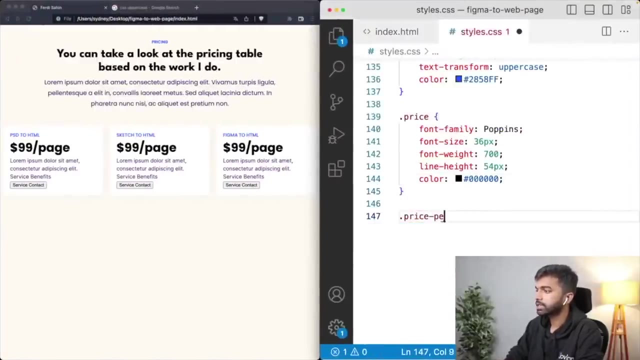 In fact, we should probably also. we should probably also have a. yeah, all the pricing seems to be same. Okay, So price per page. and then we have the span. So, into the span, price per page. let's give the right colors price per page, and let's 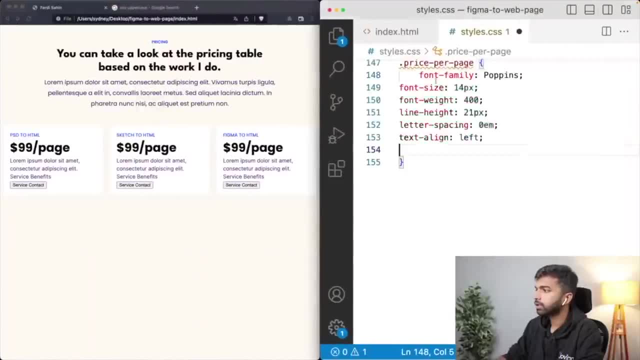 give it the color pop-ins, font weight 14.. Okay, All of this looks fine. Let's just copy that. Let's just add that. Let's reload the page. Okay, Price per page is the span or its price per page? 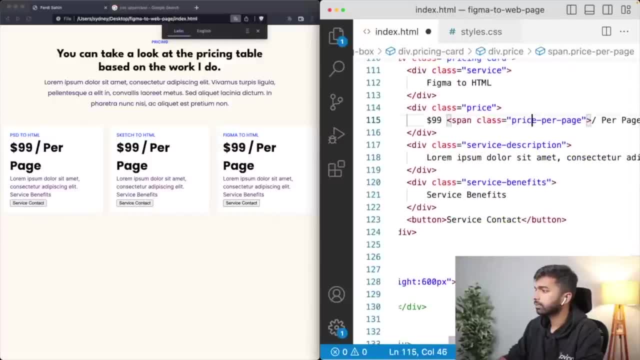 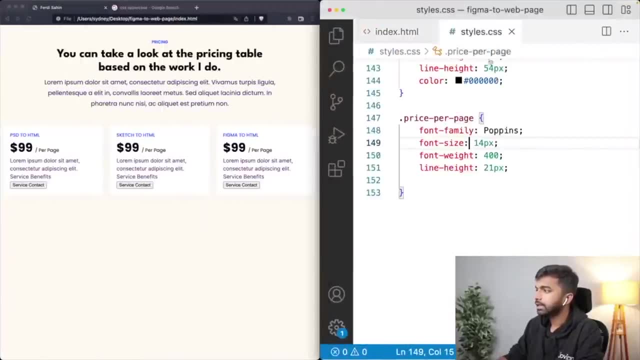 I think I made a mistake here in typing Yup, And we need to change its color as well. The color seems to be eight, eight, eight, eight, eight, So let me just change the color here as well. Okay, great, 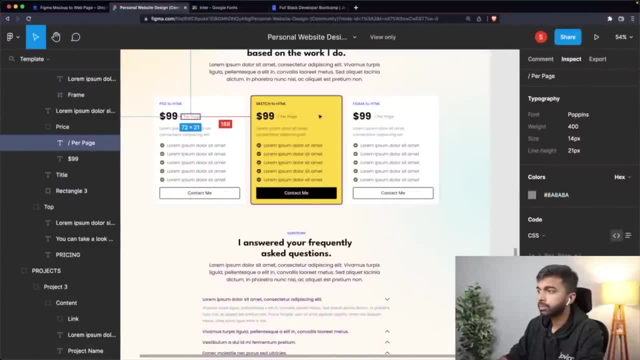 So now we have the price We got out, So price per page is done as well. Then we have this subtitle or this description, essentially. So for this description again, the font style seems to be pop-ins: 14 pixels and 23 pixels. 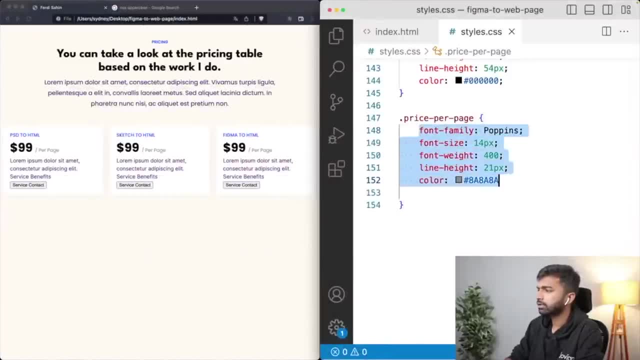 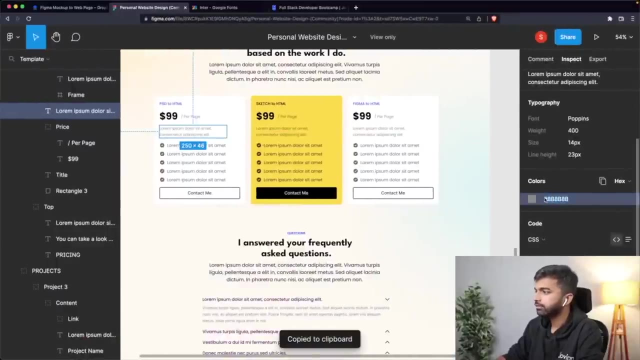 The same. I think it's exactly the same thing that we have here. So service description is exactly the same as the price per page. So service description: Yup, Okay, Yup. Eight is a color. No color seems to be slightly different. eight to be eight B. normally again, you don't use. 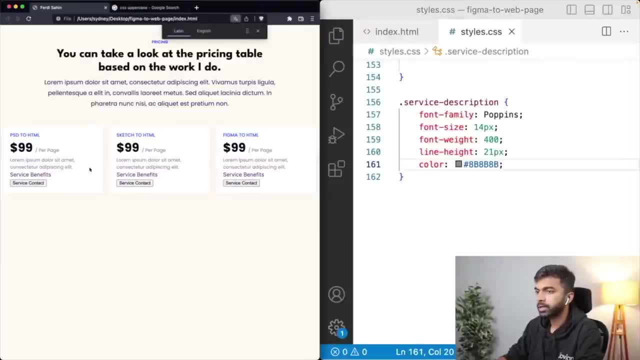 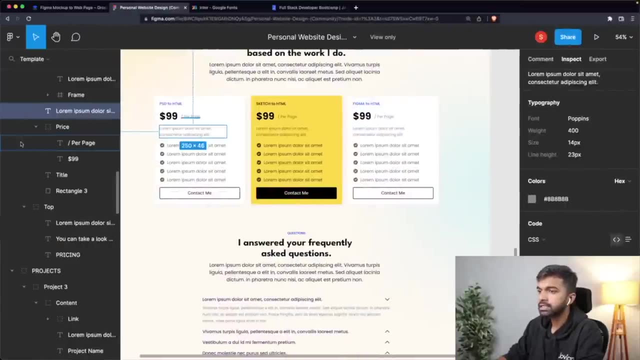 so many different colors, You have a fixed set of colors, but this particular design seems to have it, So let's just keep it that way. Let's make sure that there is enough gap. So there's a gap of eight pixels above in this case. there may not. that gap may not. 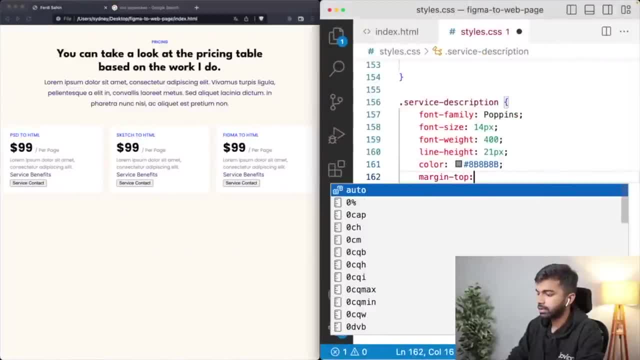 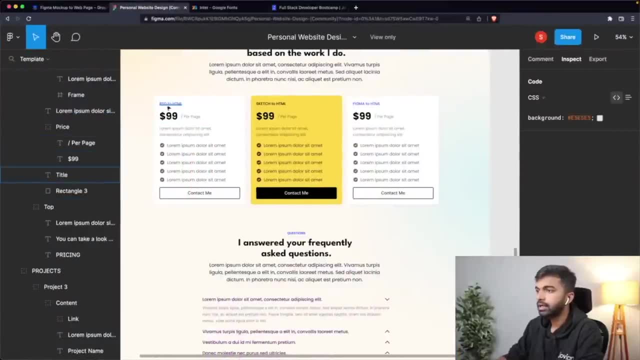 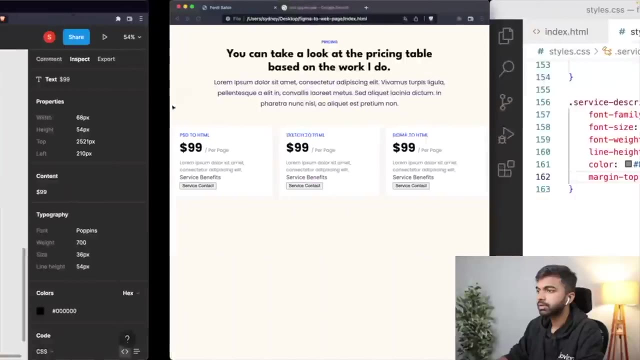 have existed. So let's add margin top eight PX And we've added a little bit of a gap, as well as expected, And there seems to be a gap between these two. So let us add that gap to what is that gap? Let's see eight pixels between these two. 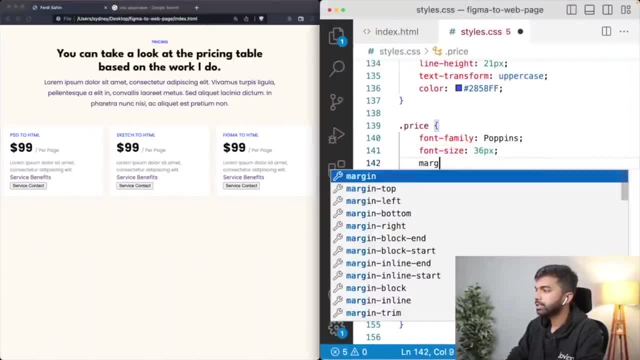 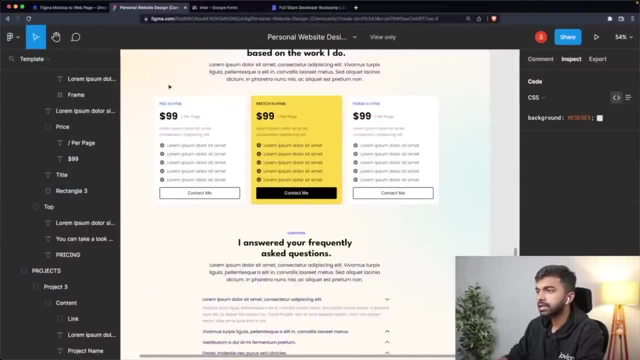 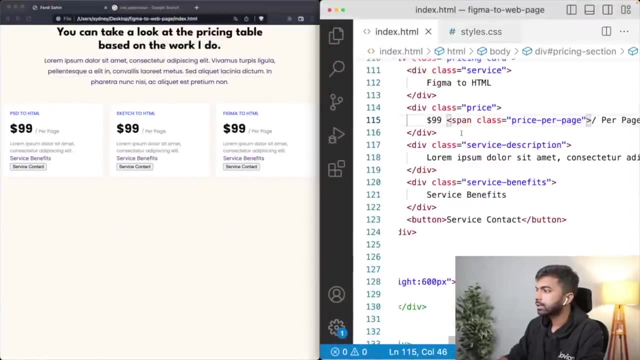 So between the price and so let's add a margin top for price of eight pixels, Yeah, So that looks a little nicer, That's again a little more spaced out, and then we have these benefits. All right, Now let me fix the benefits as a service benefits. 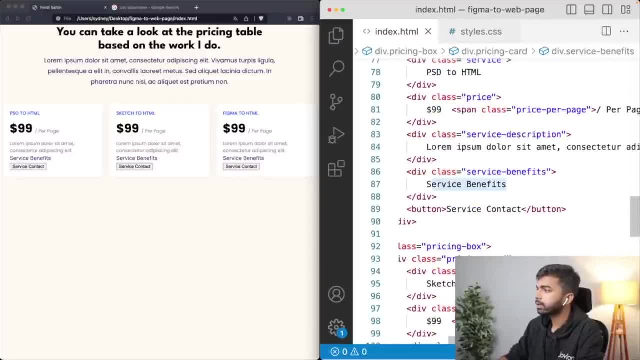 So this is going to be a list. So I'm just going to create a list here, In the first box, LI, and in this LI. I'm sorry, I'm going to use UL to create an unordered list and let's see how many benefits there are. 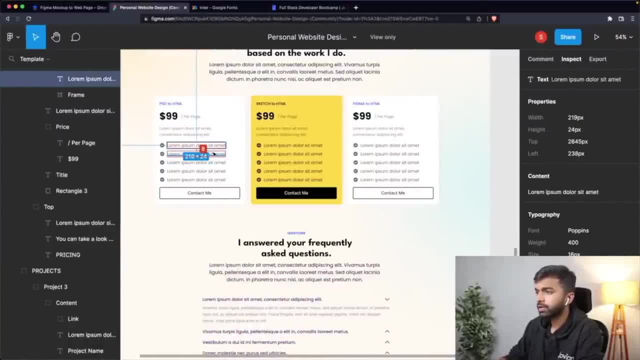 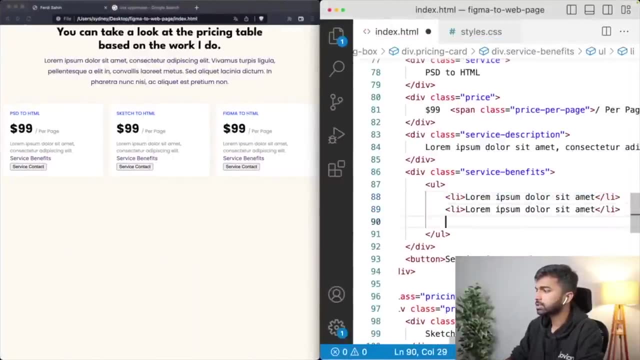 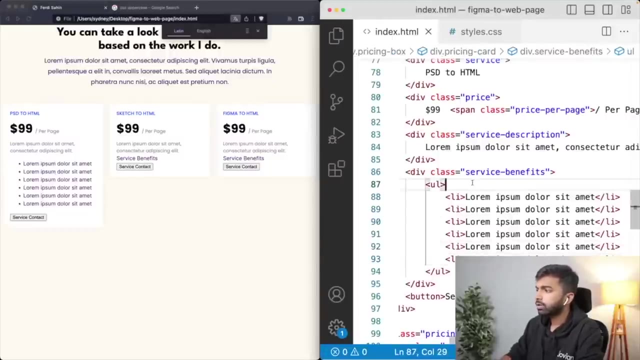 Let's add those lorem ipsum: one, two, three, four, five, six, So the benefit in each case, the value, seems to be the same, And so let's just create six copies of this. All right, Yep. Now, of course, I don't think we need this div specifically. 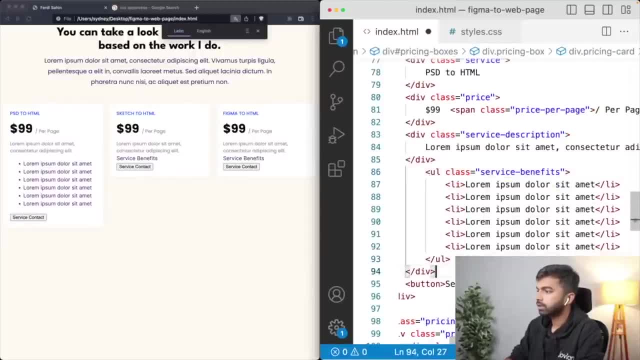 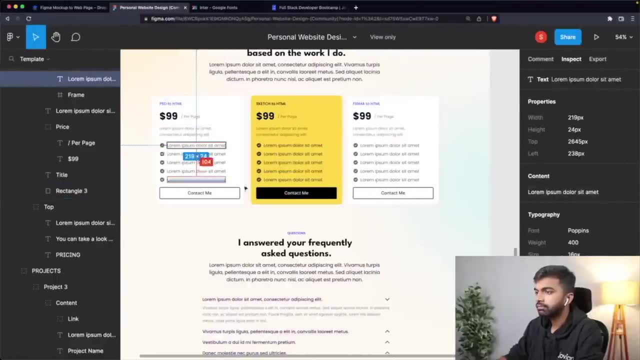 I think we can just do this on the UL itself. So let's get rid of this outer div, Let's shift this back And, first of all, I think we don't need this margin here, So it's automatically getting indented. 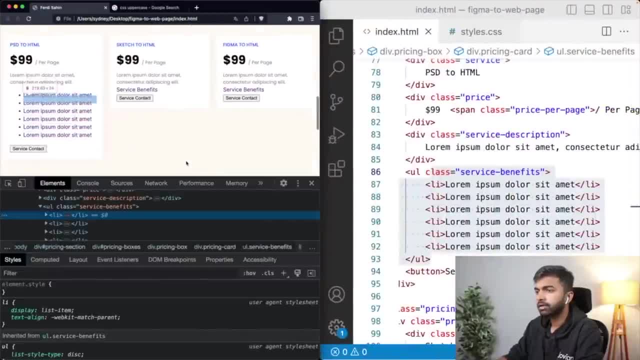 I think we don't need this indentation, So let's see how we can get rid of this indentation. Where is it? So? it is So there seems to be this padding which we can get get rid of. So service benefits. 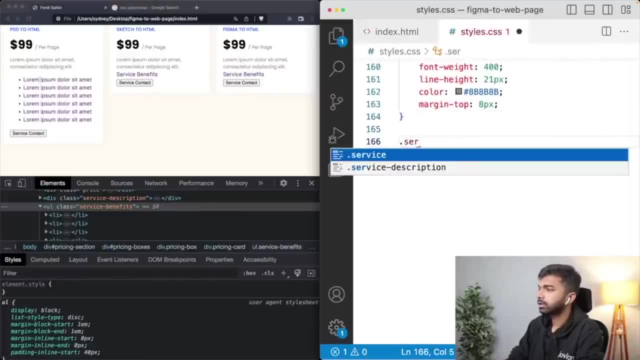 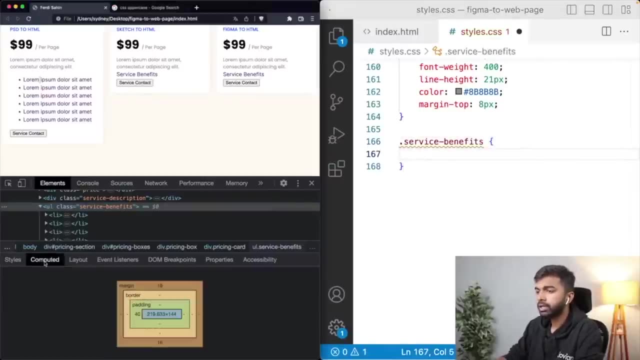 Okay, So I'm just simply inspecting it. I am then going into this, I'm selecting that particular div, and then I'm just inspecting its styles and it has a certain padding. So let's set the padding to zero, Okay. 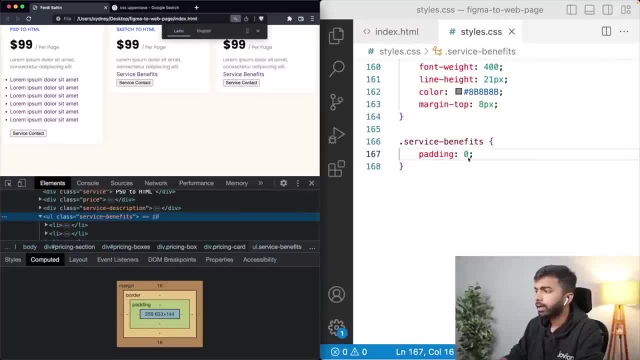 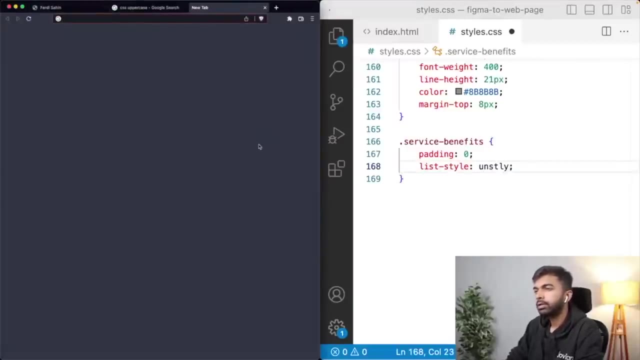 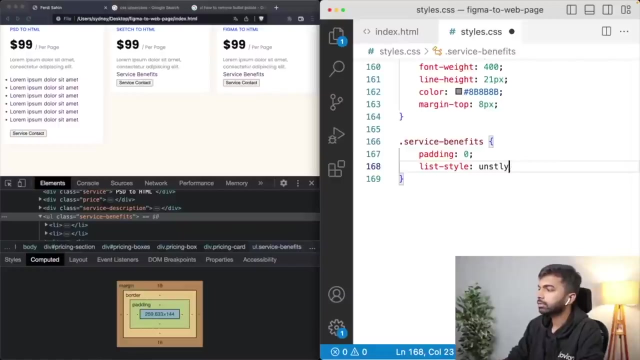 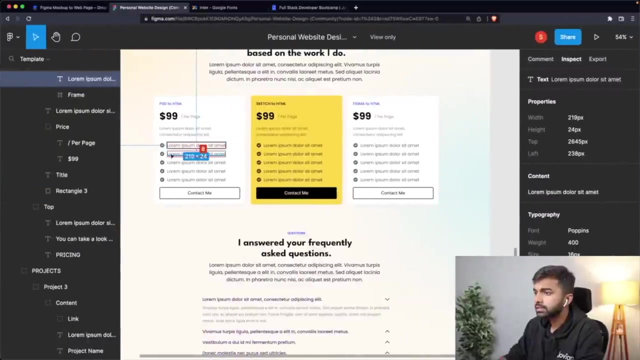 So now it is moved left Definitely. But let's also set the list style to unstyled. Unstyled or unset, or okay. UL. how to remove bullet points. list style type none: Okay. So list style type none: Okay. Then we have this check mark here that we need to somehow figure out how to add. 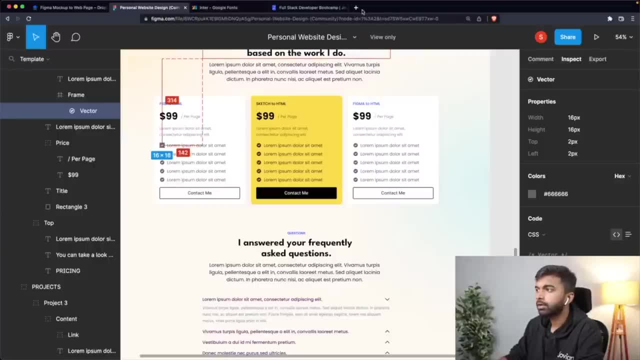 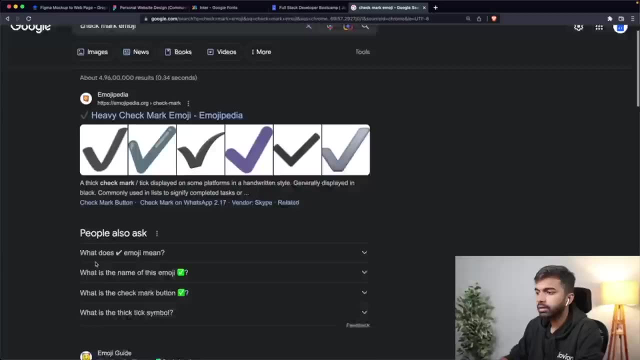 Okay, So I am going to deal with this later. for now I'm just going to maybe use an emoji. So let's just search check mark emoji, Yeah, And I'm just going to copy this emoji of over here, the check mark button, and I'm going 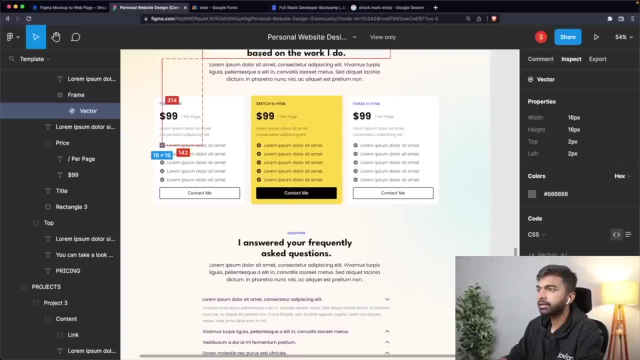 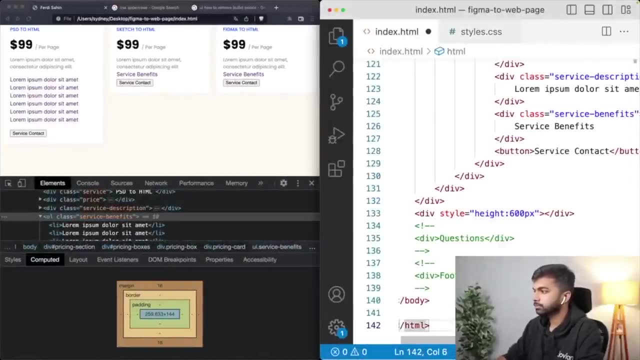 to deal with this. icons and stuff- These are things that can always be added later. So I'm just going to go in for now as a quick trick, and I'm just going to add this emoji over here. Okay, Okay, Okay. 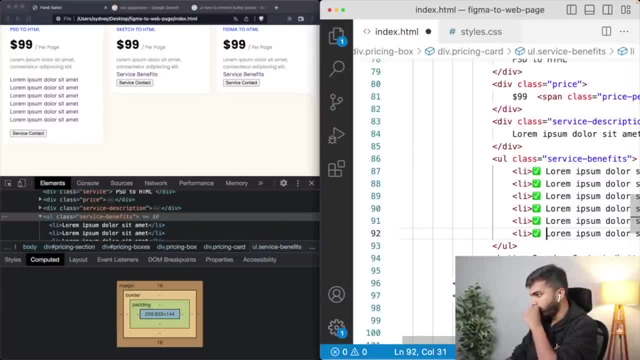 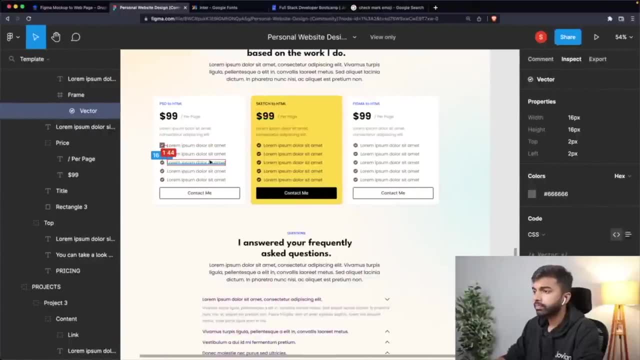 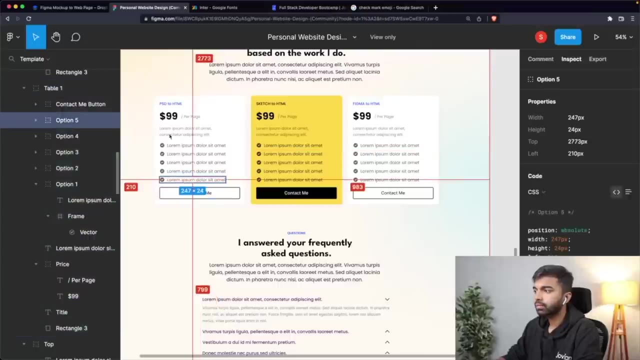 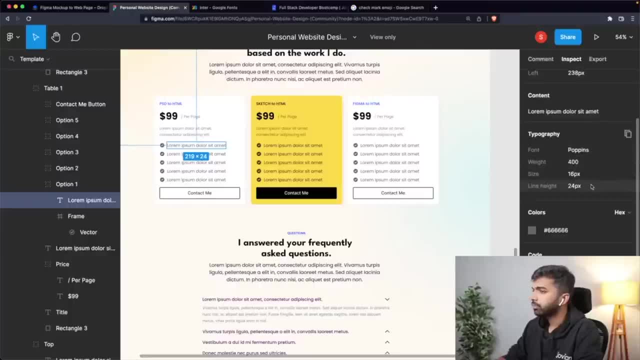 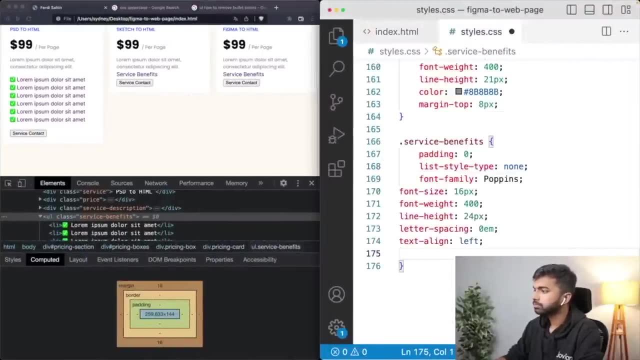 So the width, it seems to be again pop-ins, but a bigger size and a slightly different color. So I'm just going to copy that And I'm going to put that Under the font settings. So now, font size is 16, font weight is 400. line height is 24 pixels. 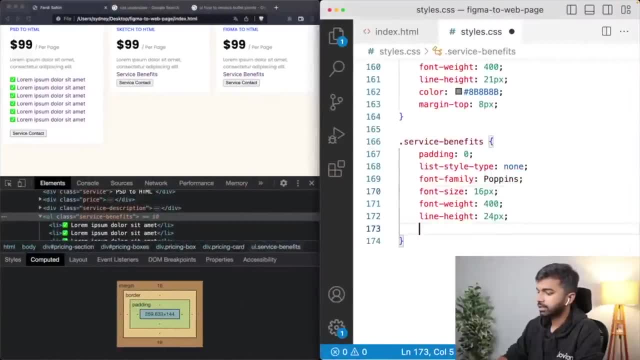 And I'm going to copy the color which is 6, 6,, 6, 6.. So I'm going to say color 6, 6,, 6, 6, okay, Yeah, And what is? I think this is looking exactly. no, this is not looking exactly the same. 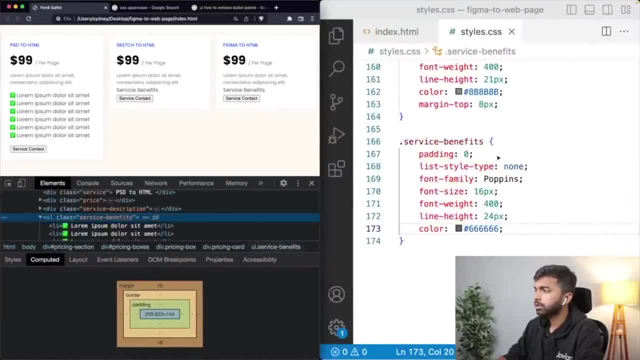 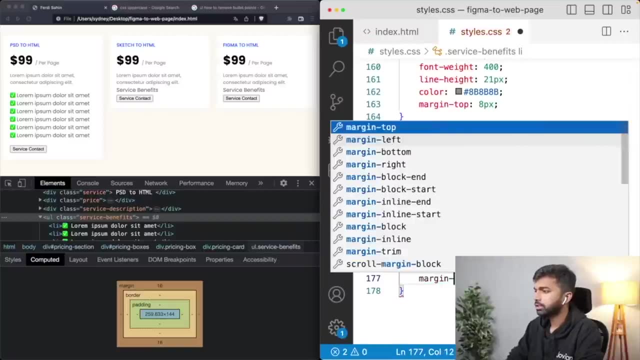 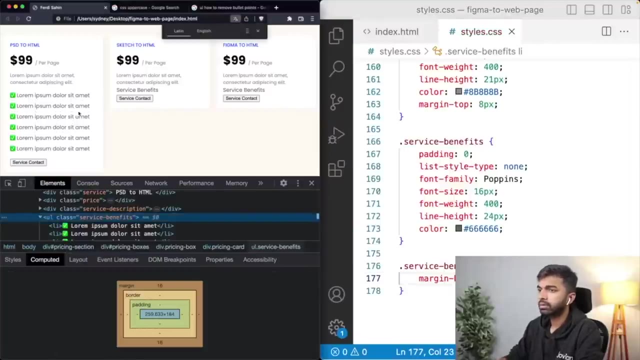 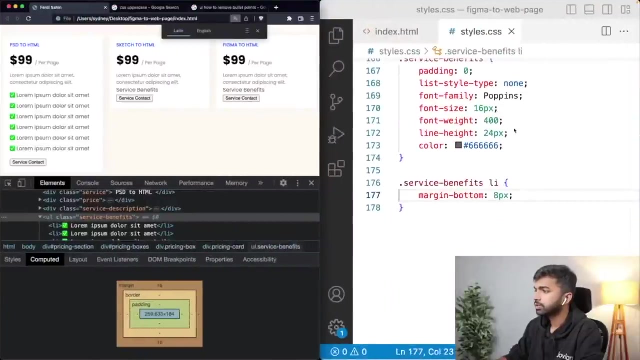 Seems like there is also an eight pixel difference between each one. So here's what I'm going to do. I'm going to say service benefits- LI margin bottom 8px. yeah, And now it is a slightly more spread out and, yeah, it looks fine to me. 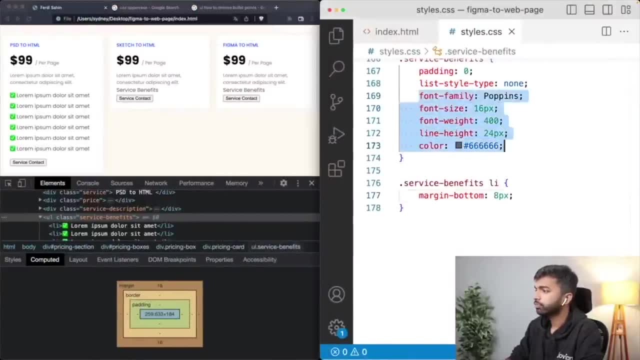 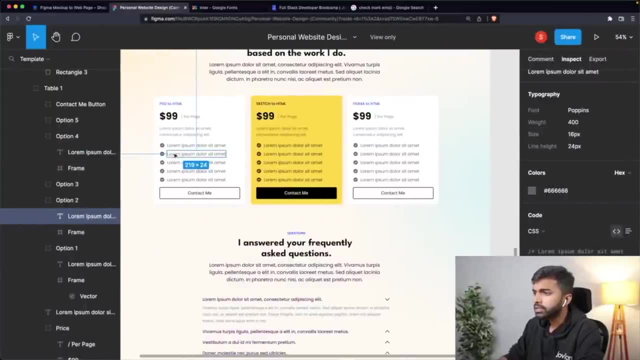 I think maybe all these, all these settings can actually just be moved into the LI itself, Right, Okay, So it's looking pretty close. weight font: weight: 400, line height 24 pixels and margin: bottom of 8.. And then, finally, there is this contact me button. 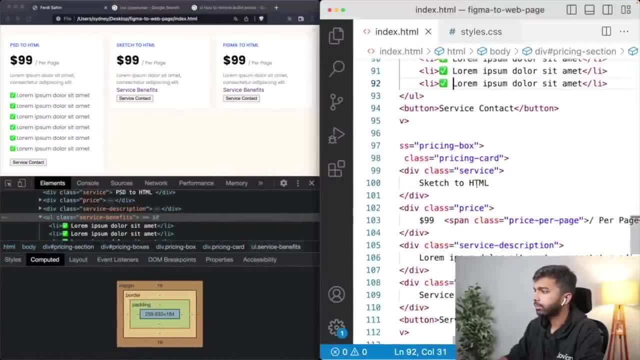 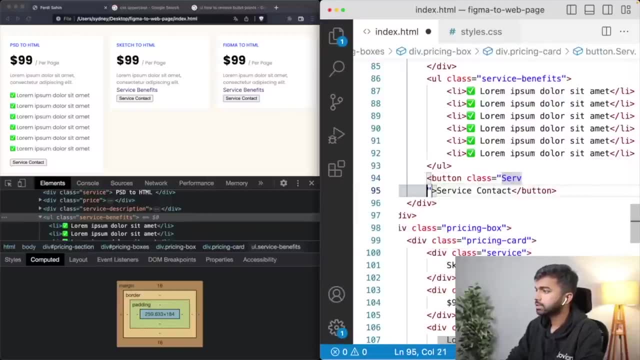 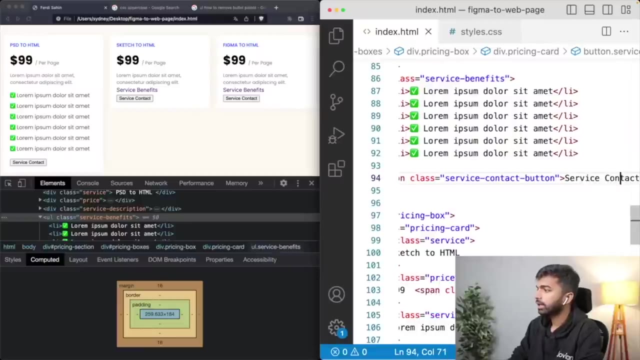 So let's add that contact me button. So this is service contact button. Let's give it a class service. Okay, So this contact button, all right, And it simply says contact me, right? I think it just says contact me. 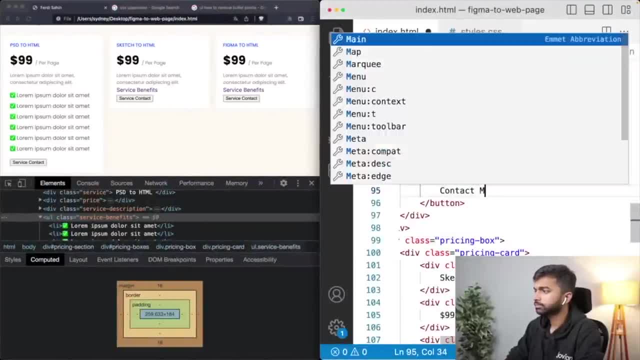 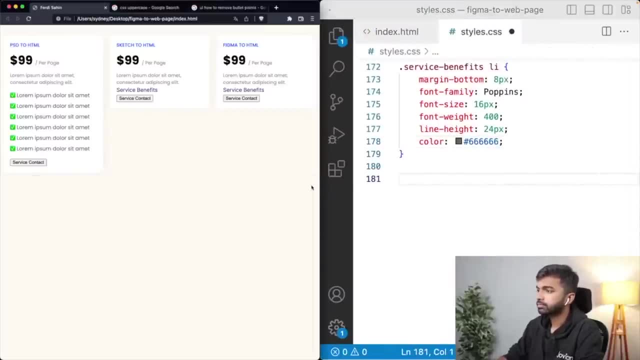 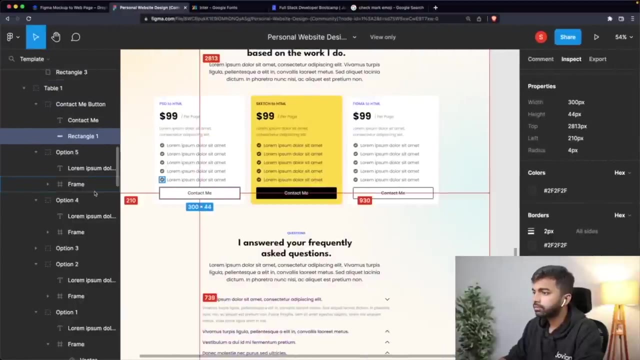 So let's go in here, Let's say: let's call this contact me and let's come back and let's start styling this contact button. Okay, Let's close this for now. So for the service contact button, first thing seems to be that there is: 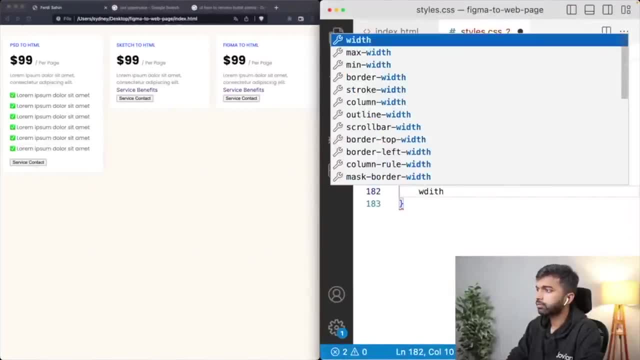 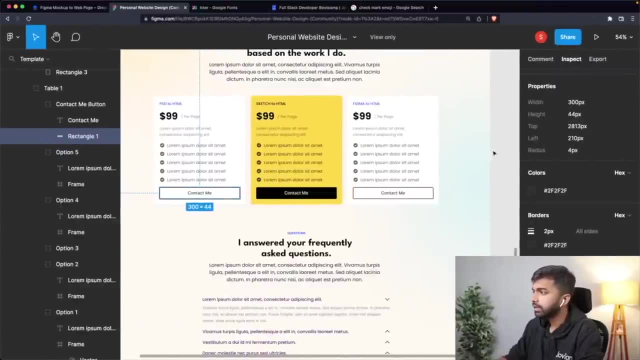 The the width is just full width, So I'm just going to set width a hundred percent so that it takes up the entire width. Then there seems to be a height, or actually we can just figure out, maybe, what is the spacing that is there within. 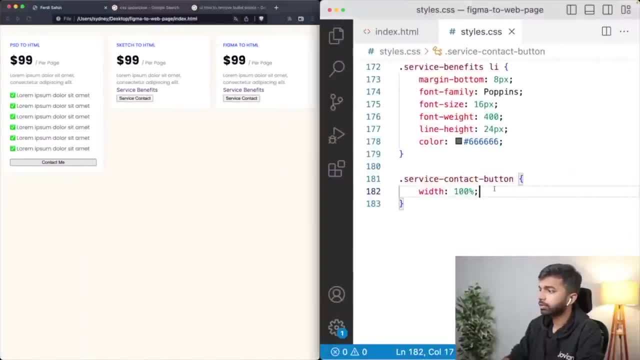 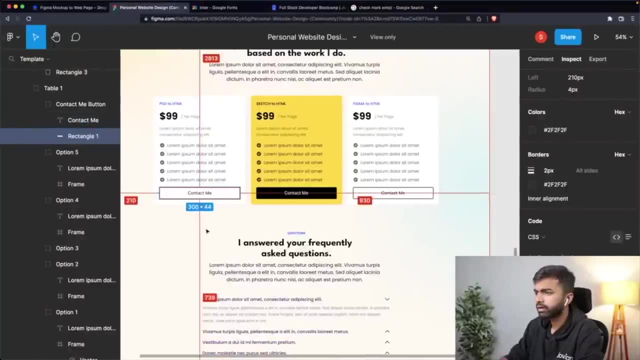 So there seems to be a 12 pixels padding at the top and bottom, So let me just put padding 12 PX all around, just to. yeah, that looks roughly similar, Okay, Does it? Yeah, Well, we can just set a height. that that could be the other thing. 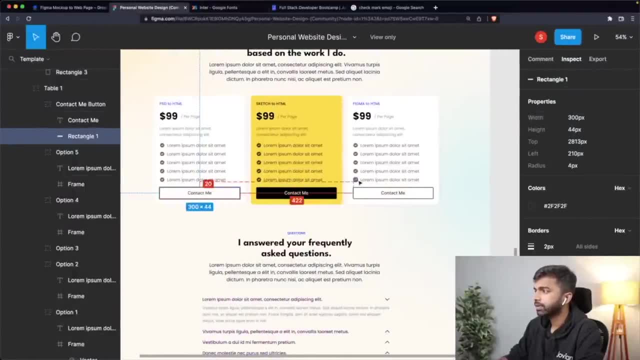 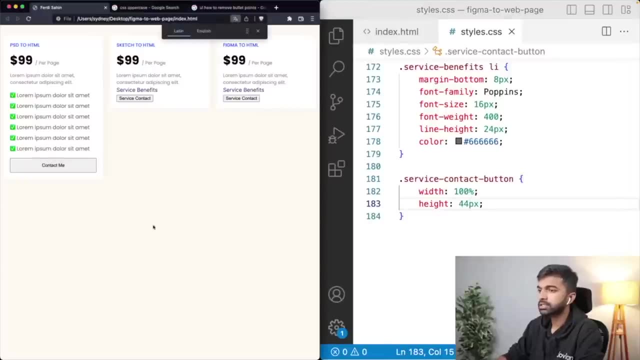 We can just set the height for the entire thing. Let's see, The height is 44 pixels, So let's set a height. So often you'll have multiple ways of implementing this. I'm just going to set the height to 44 pixels. 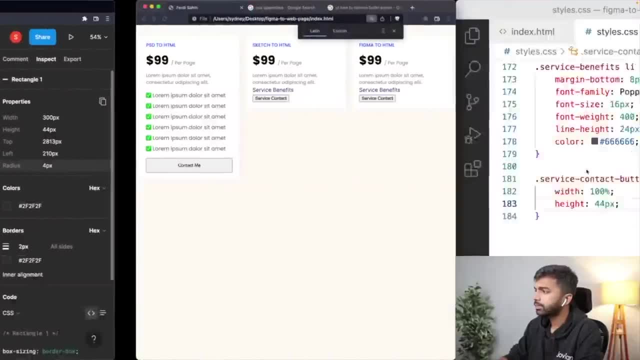 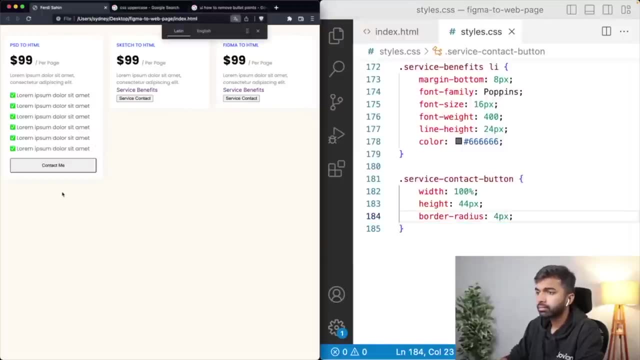 Yeah, I think it is about the same. Then there is a border radius. A border radius is 4 PX. Okay, great Border radius has been set. I guess the border width can be set to zero, or maybe one one pixel. 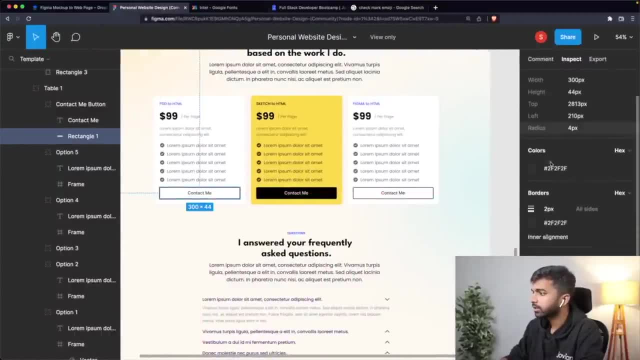 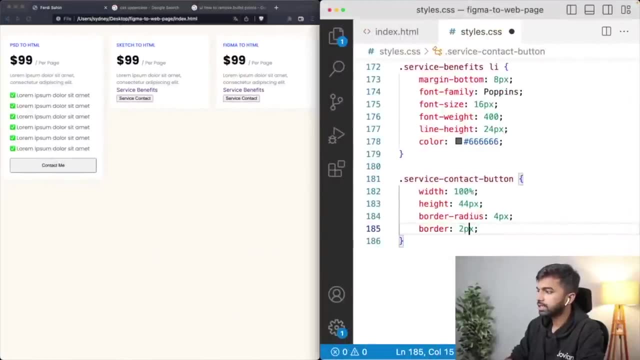 Yeah, Let's see What is the border width here: Two pixels and 2F, 2F, 2F. So border is 2 PX solid hash- 2F, 2F, 2F. That is a color. 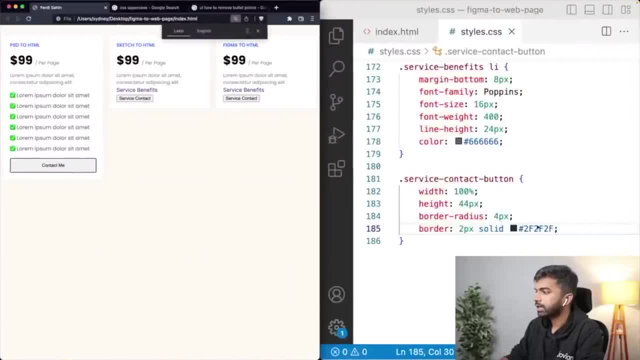 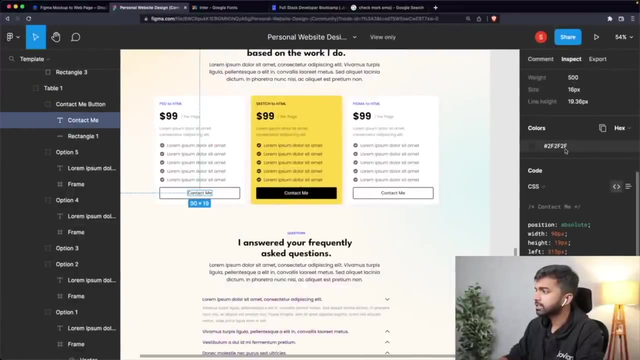 Then there's a background color. The background color in this case simply seems to be white. So we can just say background color FFF, FFF, which is just white. Okay, Now we need to actually add some text colors. So the text color seems to be 2F, 2F, 2F. 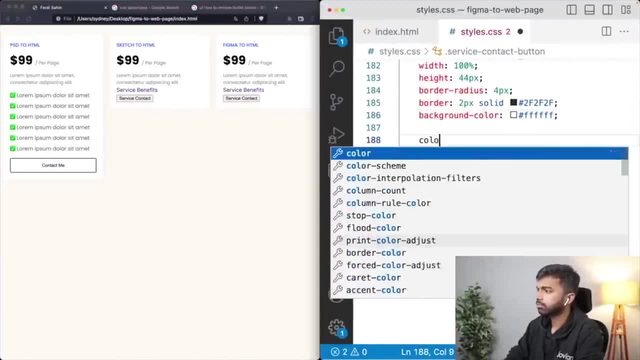 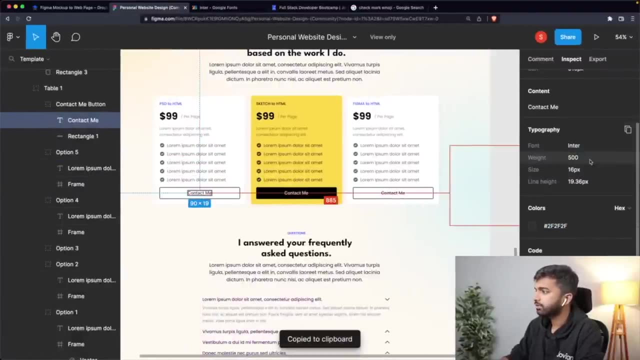 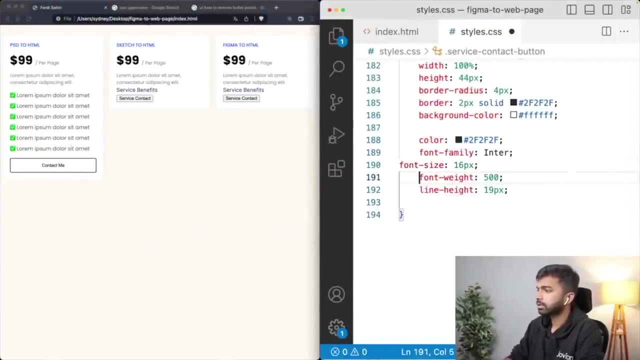 So let's add that text color. Okay, Then let us add the text size, or the text seems to be: inter weight 516, line height 19.36.. Let's add all of that in here. So, even though there are two different elements on Figma, on our, when we are creating the 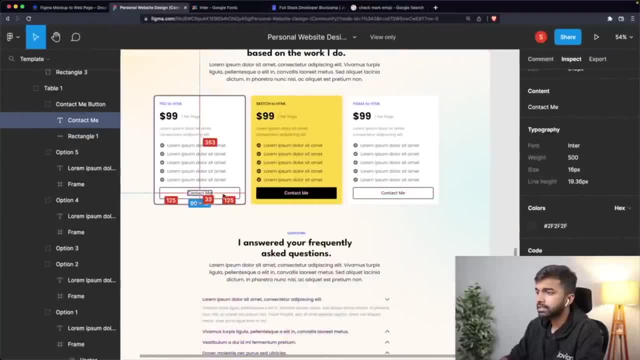 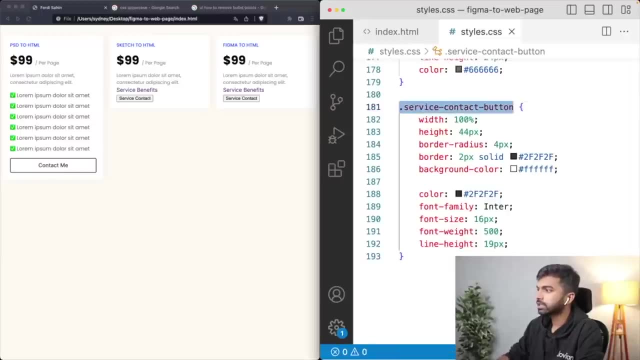 button. it's just this one thing, All right, And that's it Now. of course, we may want some sort of a hover state here, So you may want to say something like this, where, when we hover over the service button, 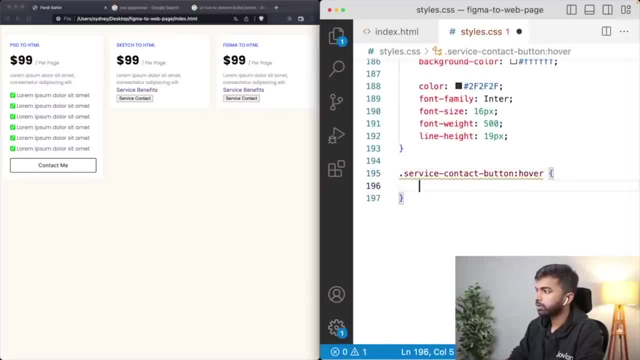 some of the things reverse. So when we hover over the service button, maybe the background color could become 2F, 2F, 2F, Okay, Okay, Okay, And the text color could become could become white. So that is F, F, F, F, F, F, but text color is just color, right. 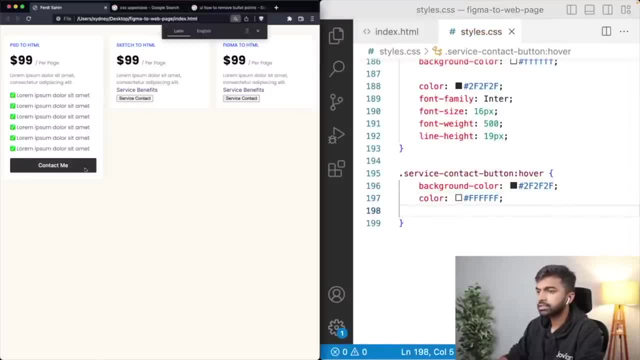 And maybe you also want to turn. let's see, I think this should do it. Yeah, Maybe we also want to turn this cursor into a hand button So you can say: cursor pointer. This is again. This is a common thing that you will often end up using. 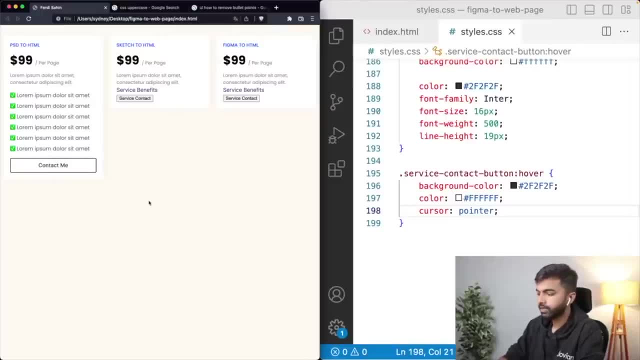 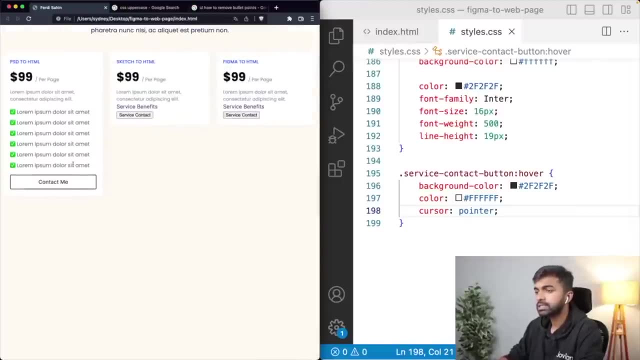 It turns into a hand button over here, right. So now you see if I zoom in a little bit. so you see, now we have this contact me button and now we have these preferences, and now, of course, we can copy that over to the other. 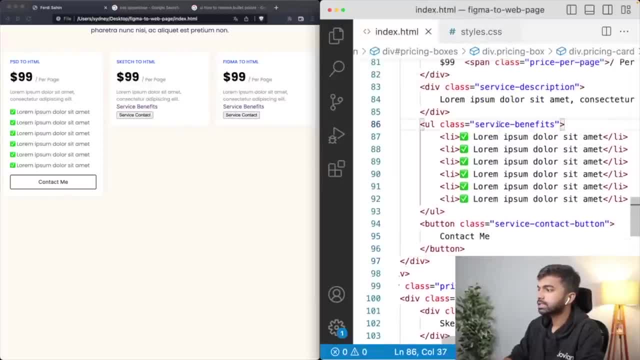 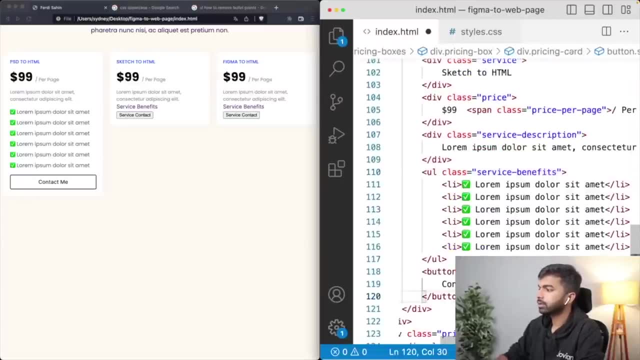 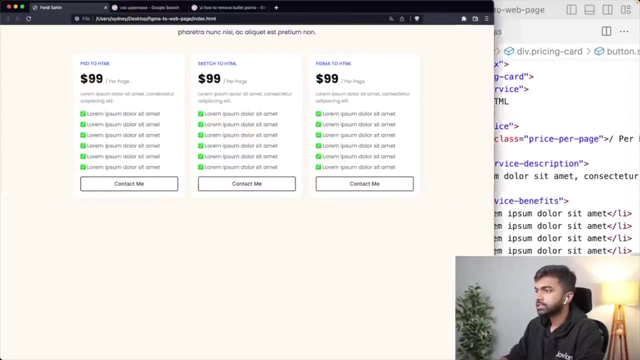 ones as well. So let me just copy the service benefits and let me copy the contact me button. Let's copy it over to the second one. Let's copy it over to the third one. Okay, So now we have a pricing section. that is more or less what we expect. 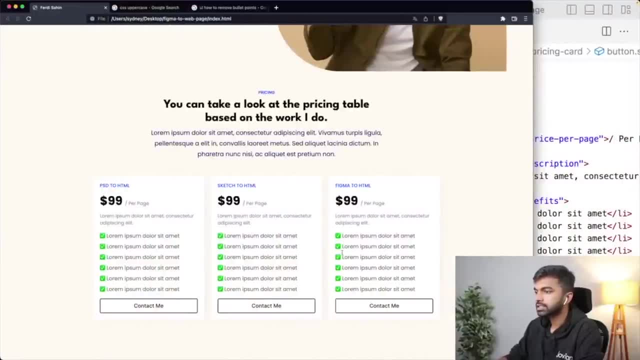 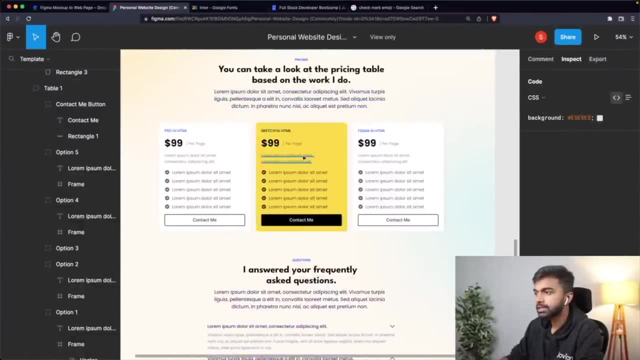 So this is what the pricing section looks like here, and this is what the pricing section looks like here. Now, of course, the second pricing section, the sketch pricing section, seems to have a yellow background and a few other things. So that is something again we may have to figure out how to do. 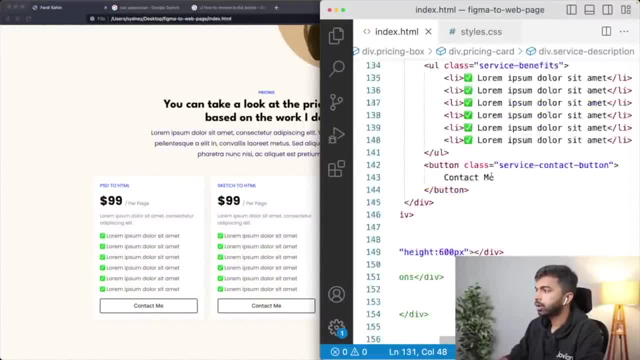 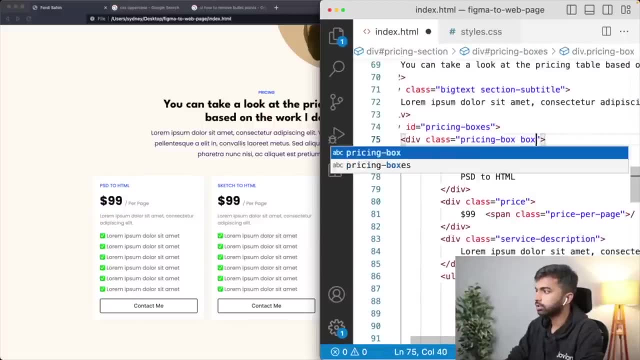 And I'll show you the quick way to do this. What do you do is go into that second box in Yeah, So this is the Yeah, Yeah, So let's add it. Let's add box two here, box two, pricing box, box two, and into box two. you can actually 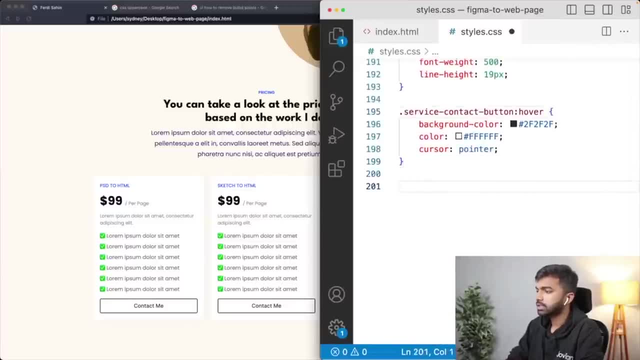 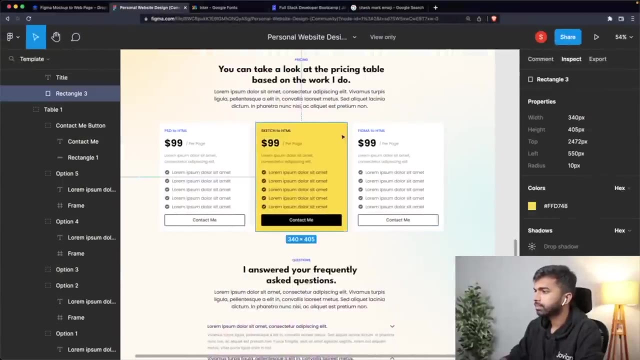 go in and add specific changes So you can say, dot pricing box, dot box two, So when it has both of these, both of these classes, in that case we want the background to be yellow, which is just this, this color over here. 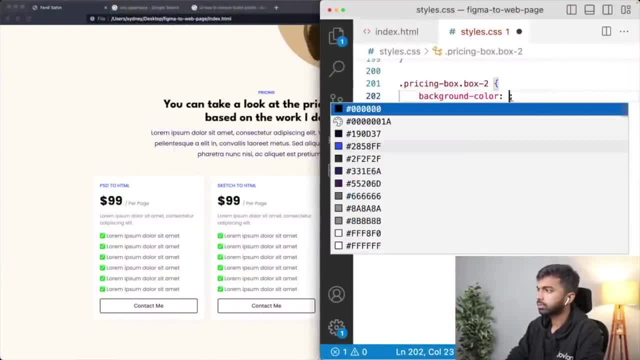 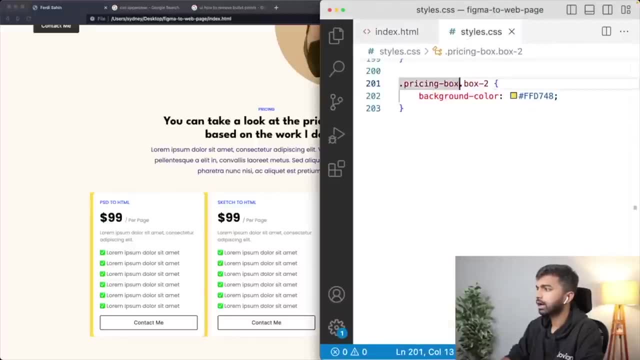 So I can change the background color to that. Okay, That's probably not added to the right thing. I think it's pricing card that we need to add to, And let's let me just call it card two instead of box two. 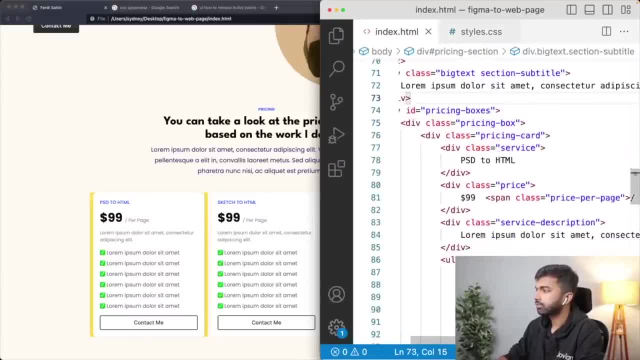 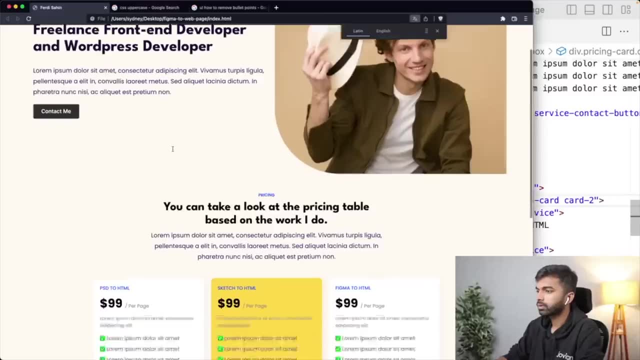 So let's get rid of that, and I should be adding it on the second one. So this is the second pricing box, and in the second pricing box let me add card hyphen two. And now you can see that it has changed to yellow color. 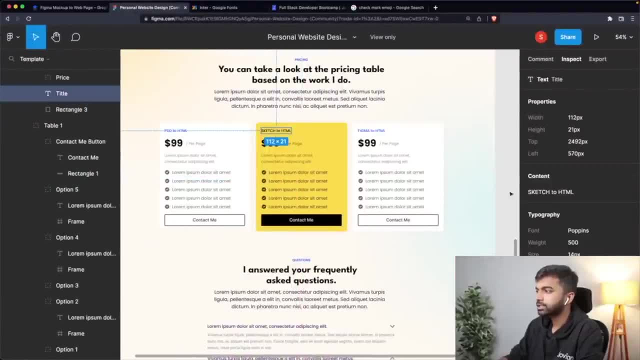 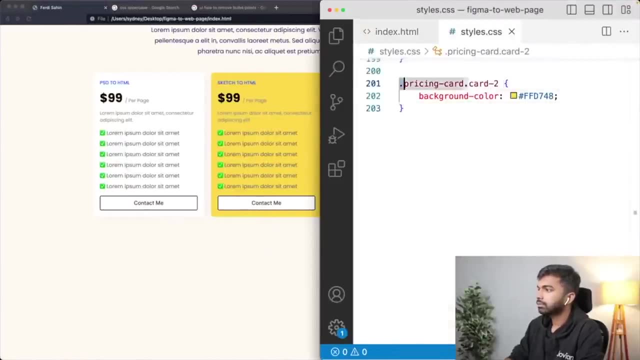 Yeah, So let's quickly modify these styles as well. So here it is, just sketch to HTML is just black. So I'm going to say that within: I don't need this. So I'm going to say that within card two: if I have a service, then the color should. 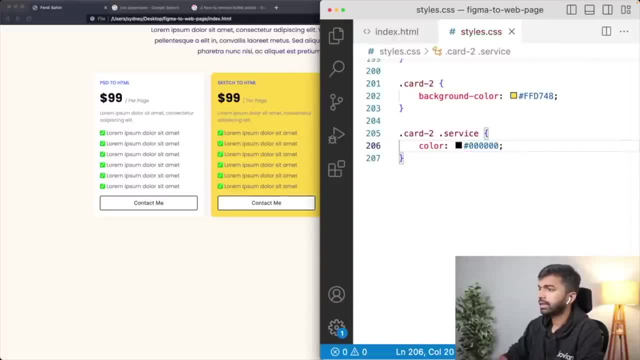 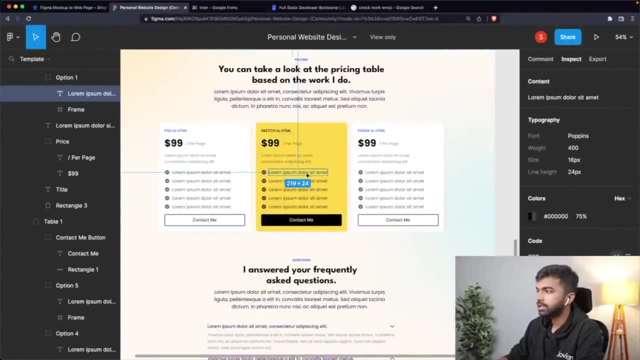 be black. Let's reload that So the color has become black. Then everything else looks fine to me. Maybe this may need some change. The color here is also black, or but 75% black, So we can kind of copy that. 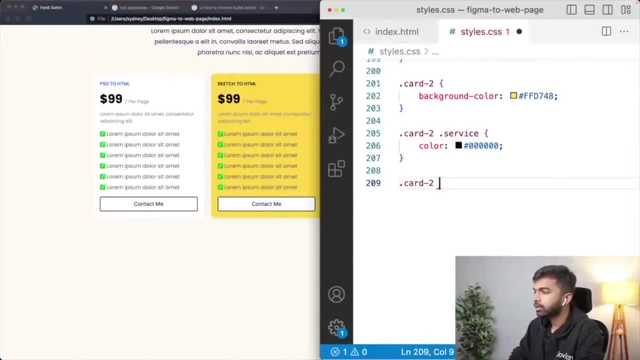 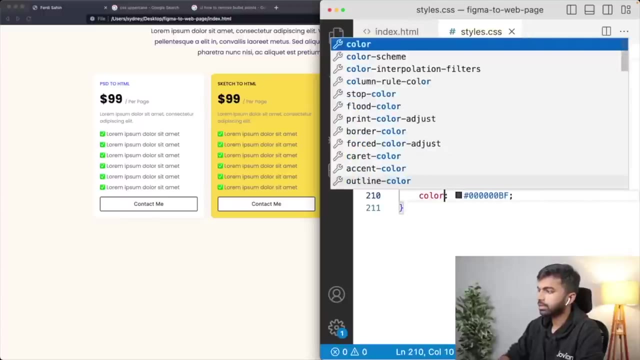 So within card two if I am looking at a list item or specifically if I have service benefits, or let's just do that within card two. if I have a list item, then I want its color to be that and I can just change the color for that list item. 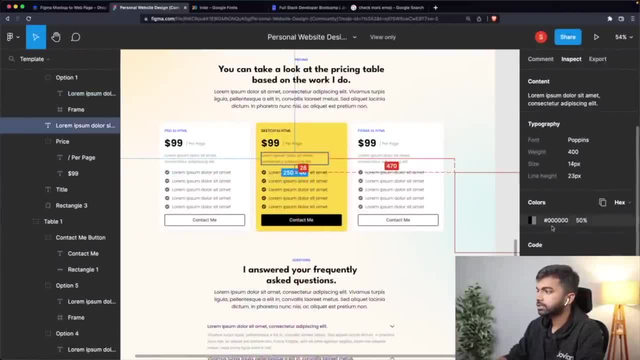 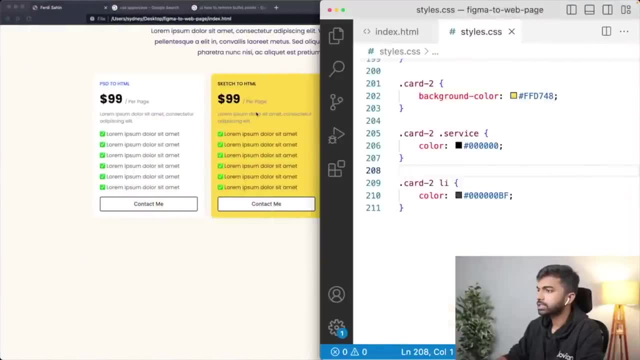 And similarly, I can change the color. Okay, So I can change colors if required. So it's 50% here, 50% black here, So I can just copy this color and I can apply that to what is this? well, I believe this. 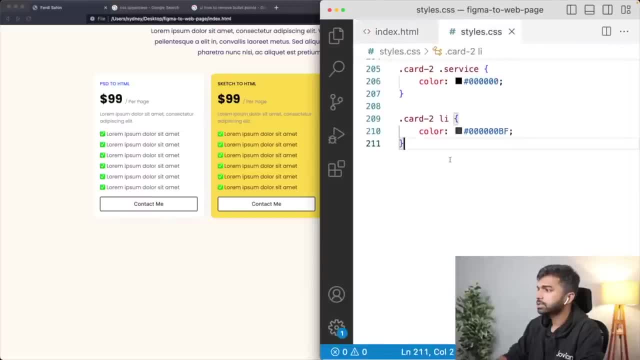 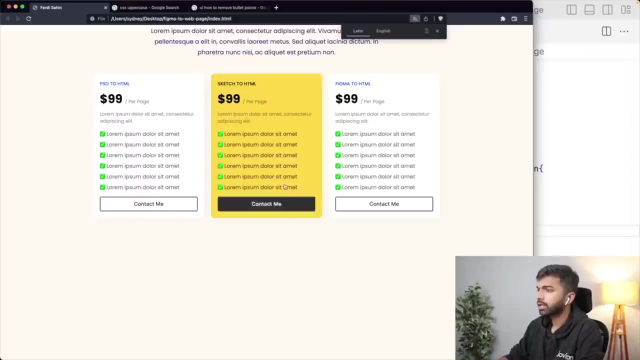 is service description and price per page. So within card two, if I have a service description, then the color is that. So you just add this additional selector. And within card two, if I have this price per page, its color should also be that right. 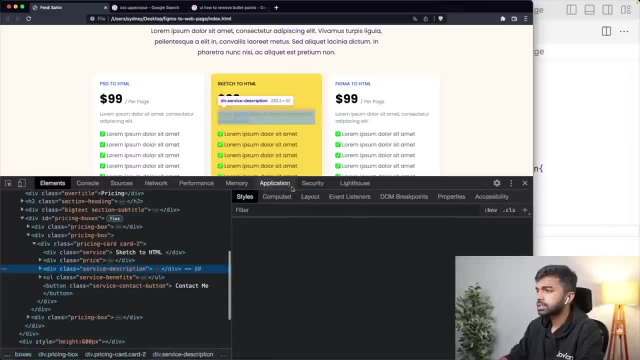 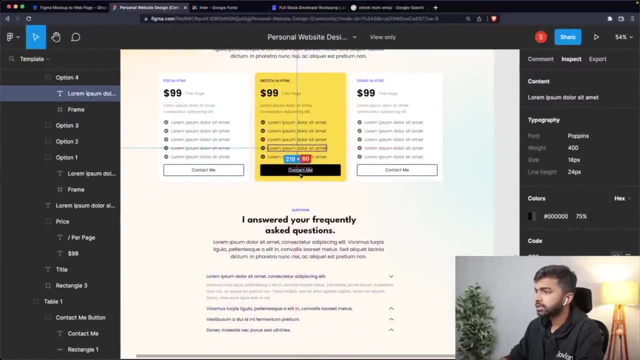 And now we have- I believe we have- the expected colors. You can see here that I can check that. card two: service description is the selector for it. What else? Well, we have. this contact me is black and white, so it's the other way around. 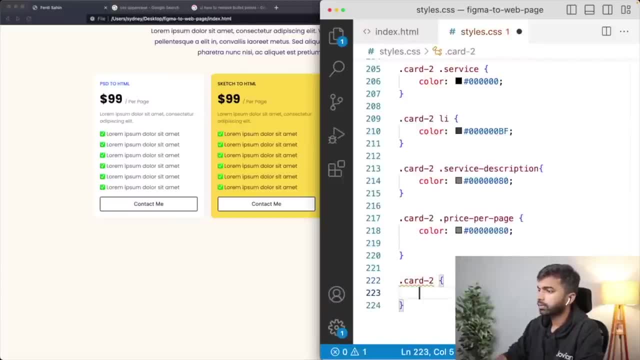 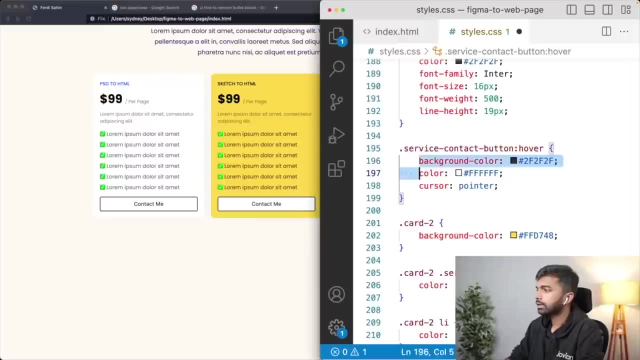 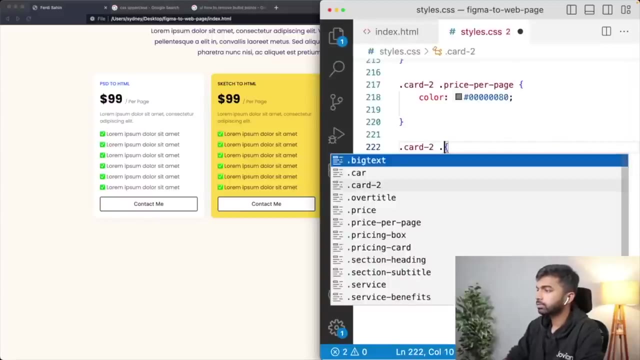 So within card two. Okay, So within card two we have the only changes that background color and normal color are from the hover state and within card and of course this is for the contact button. So service contact button and let's flip the styles for the hover state. 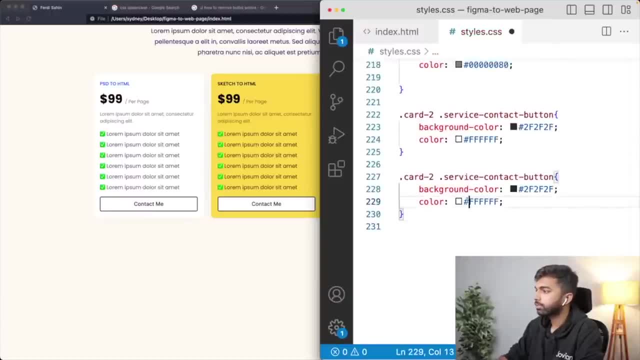 So when we hover over it, we want it to be the other way around. So the color is going to be FFF. Okay, Okay, Okay. So the other color here is going to be 2F, 2F, 2F, okay. 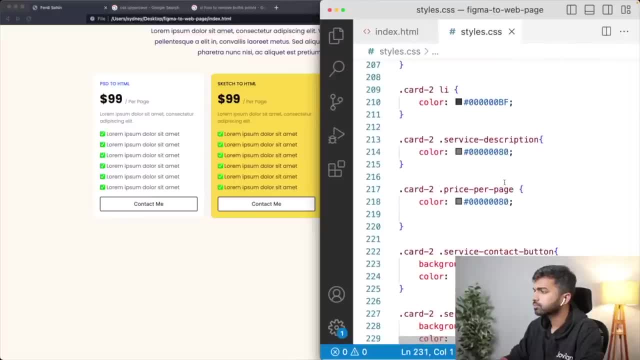 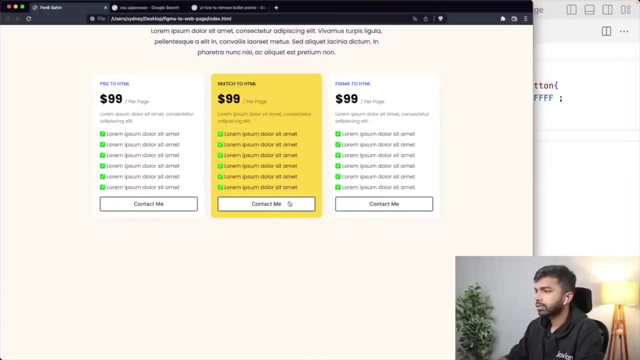 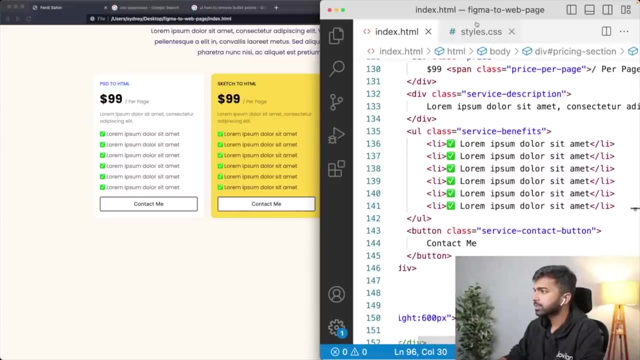 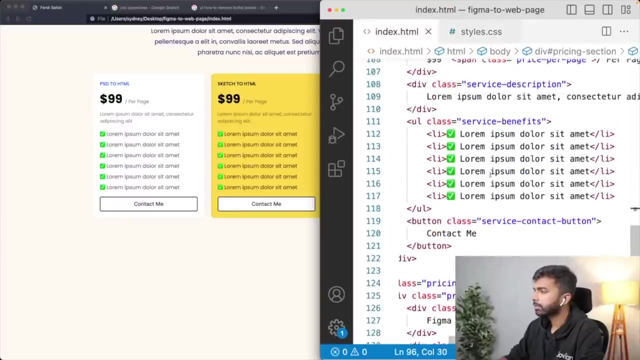 Service contact button. well, that doesn't seem to have applied. We can just give it. we can just give that button a specific card or a specific Yeah. Yeah. So let's just give that button a specific uh class here. 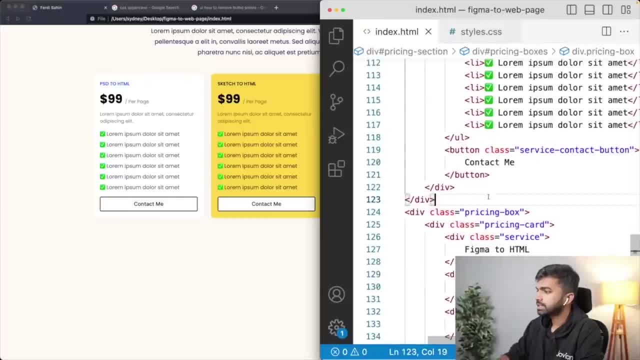 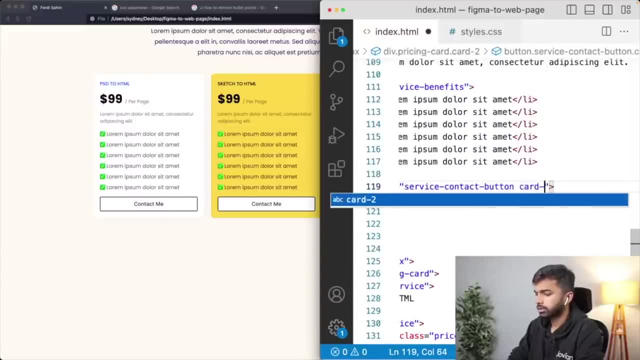 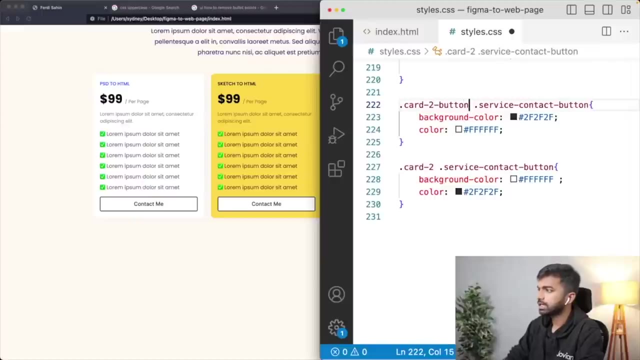 So service contact button for card two. Let's see card to button, card to button. So let's just do that. So we don't need this multiple selectors, We can just do card to select it. So, depending on what you want to achieve, sometimes you may have to come up with uh. 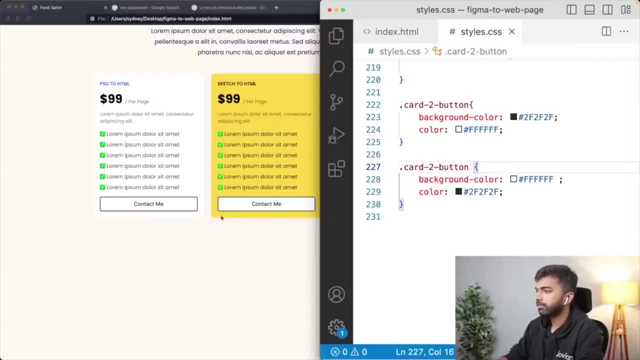 like specific classes, But generally speaking, it's with a bit of experimented experimentation You should be able to figure it out. Oh, oh wait. I think I understand what the mistake I made. I did not put the word hover here. 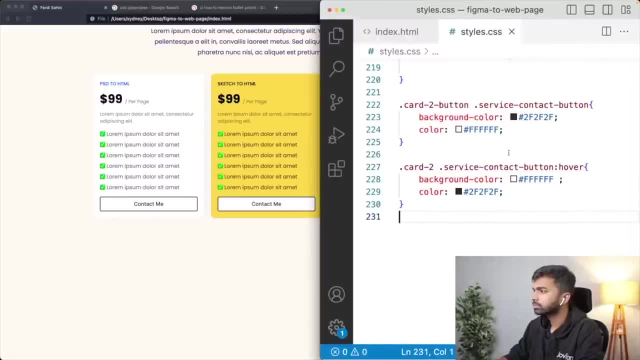 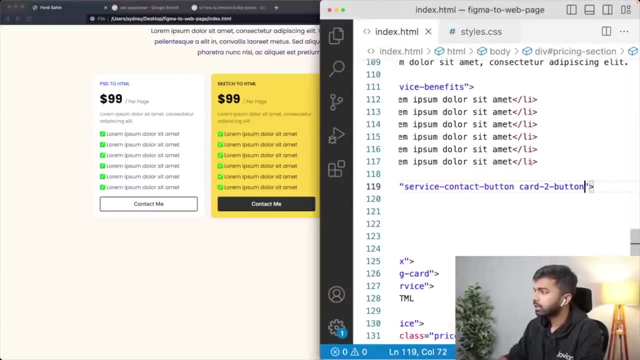 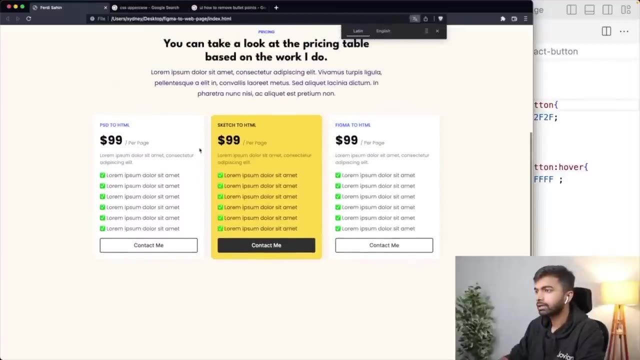 Yeah, that should do it. Card two: Yeah, that, that does it. So now we don't need this card to button class. So you'll often make these kind of silly mistakes when you are working on CSS, but this is looking good. 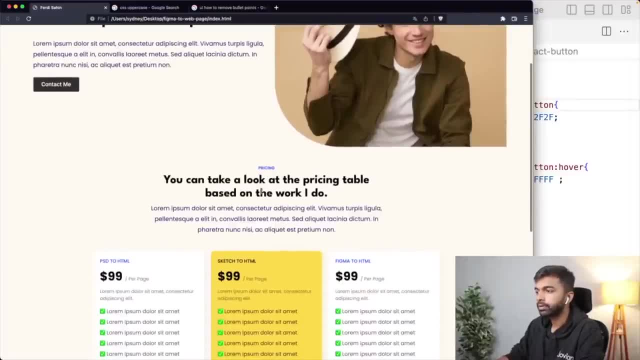 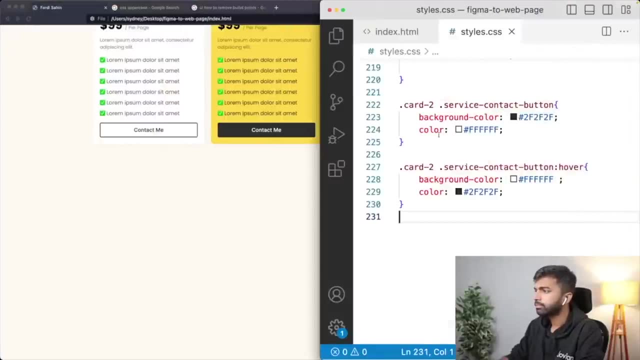 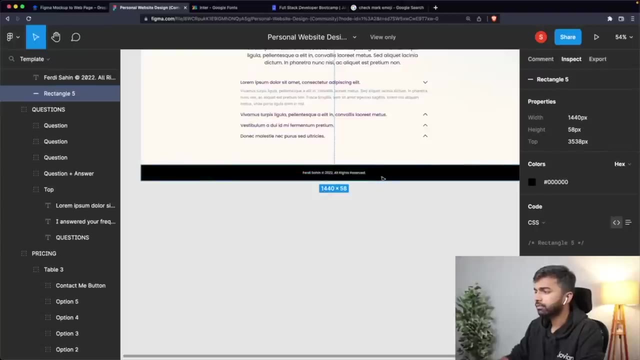 So now we have this Ferdy Sahin freelance web developer, pricing, and all of this is fine. Let's maybe add the footer as well, which should be very quick to add. So the footer is just as black band which contains a which is of height 58. 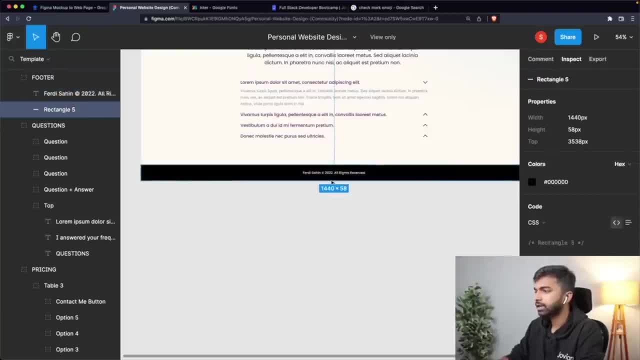 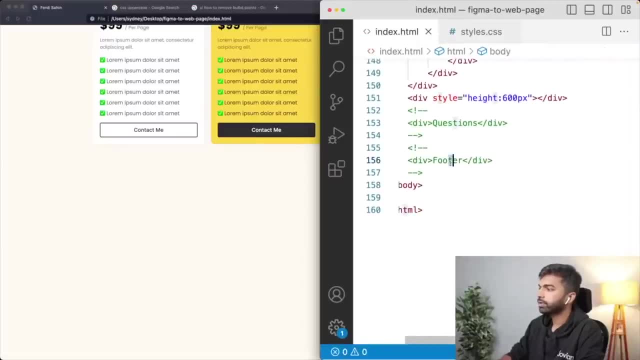 pixels, or which basically has some text and it has like a 20 pixel padding internally. So let me just add the footer And I think that'll just complete the page for now. So let's go here, Let's go here and let's give this the ID footer. 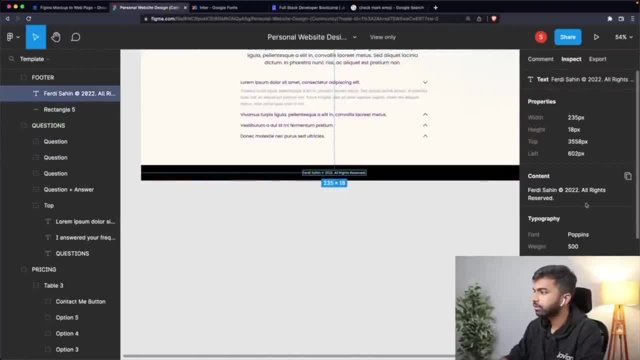 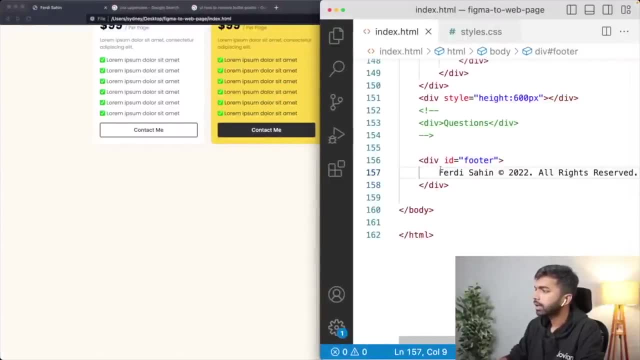 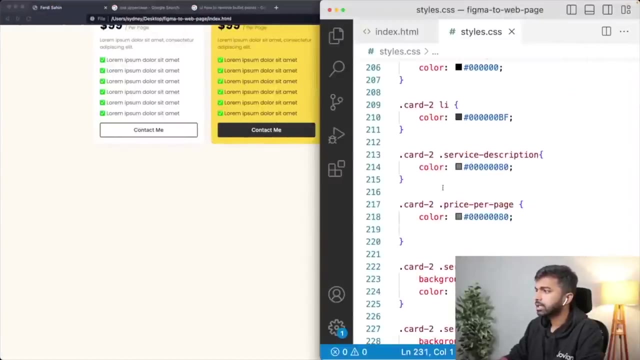 And this footer has some text. The text is simply Ferdy Sahin copyright. So let's go in, let's put in the text here and let us just give it some styles. So let me come back into indexhtml, Oh sorry, into stylescss. 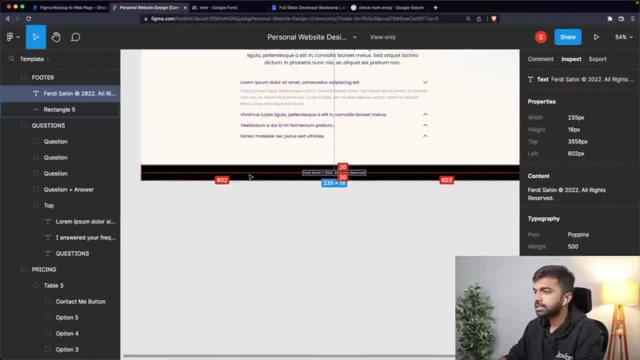 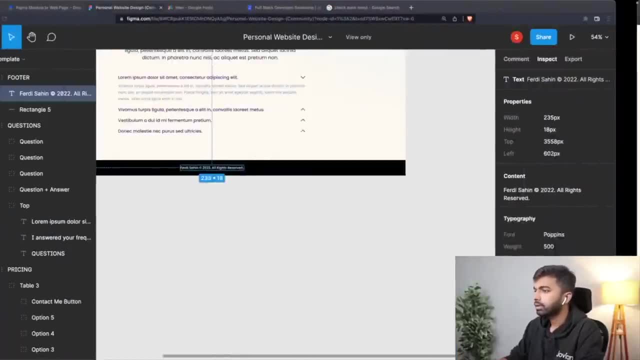 And let me go into footer. So the first thing with the footer is it. it occupies the entire width of the page. So I'm just going to give it width a hundred percent. Then I am also going to text align center. So I'm going to say text align center. 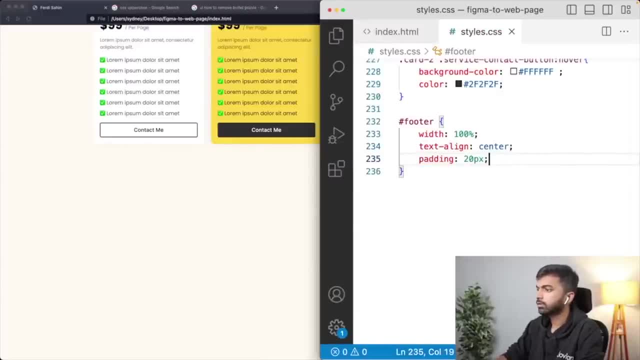 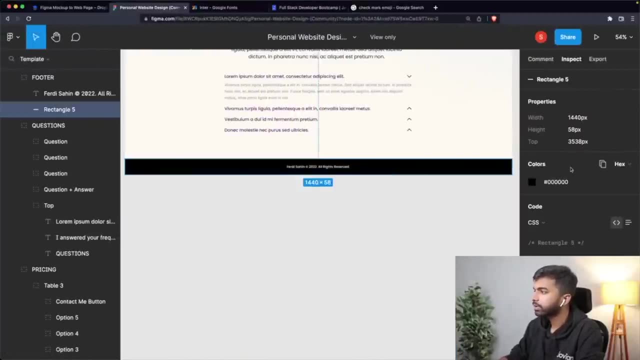 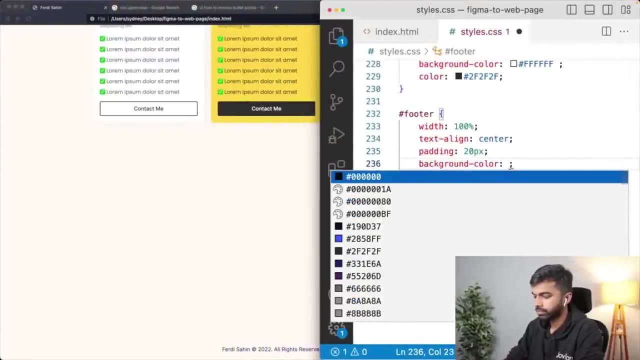 I'm going to add a padding of 20 pixels, 20 PX. So yeah, now we have that, We of course have to add a black background. Do it So? 0 0 0, 0 0.. Uh, so let me add a background color: 0 0 0. 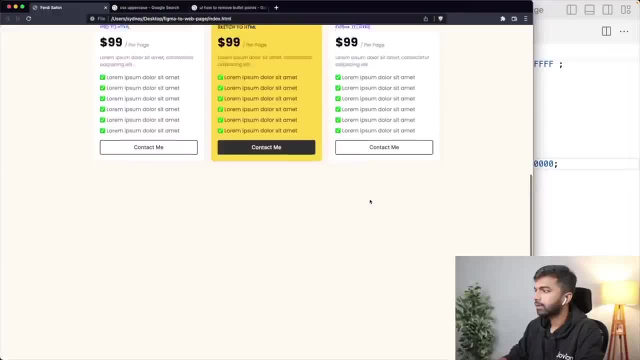 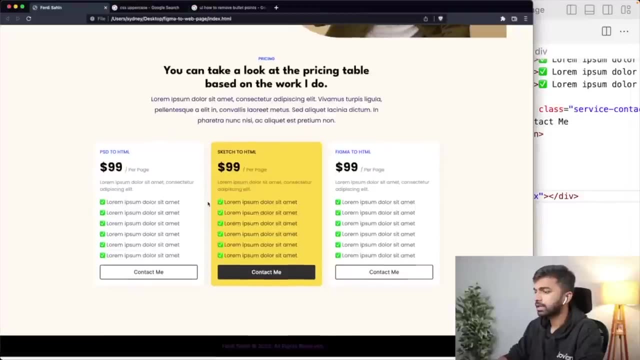 Okay, Let us change the text color over here. Um, I think I'm going to get rid of that additional div. I had, or maybe reduced its height to just a hundred pixels so that it's a little closer and you can see things more easily. 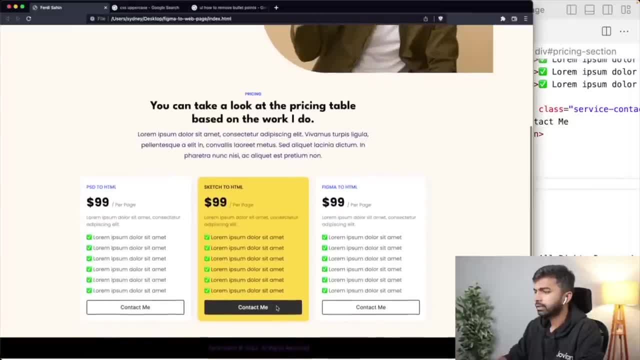 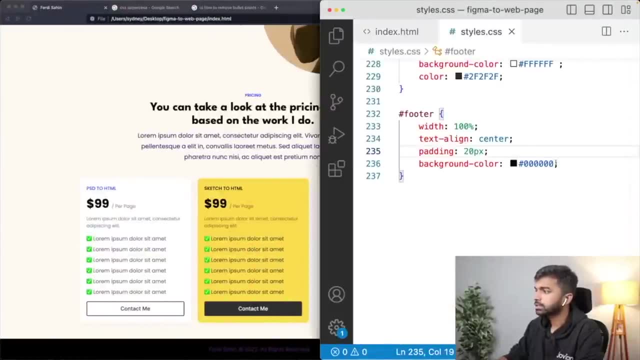 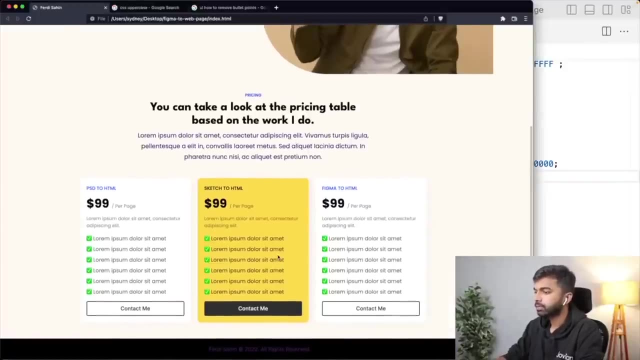 Oh, we can just get rid of it completely. Yeah, Um, let's add maybe a margin top to it so that it's not too close to the content. So I think the margin top of 48 pixels should be fine and let's change its color. 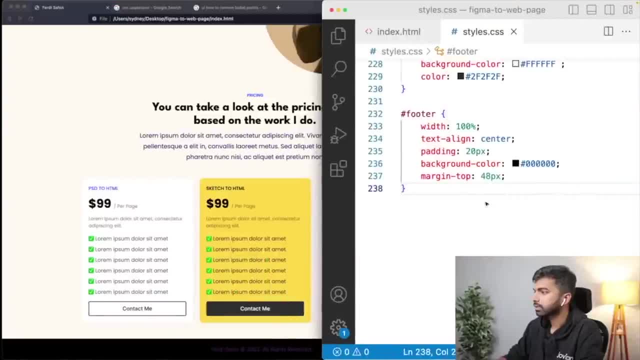 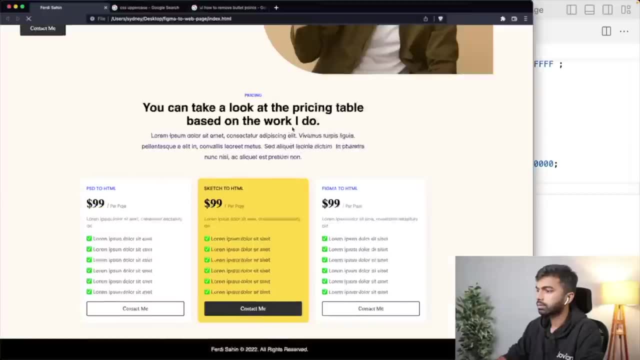 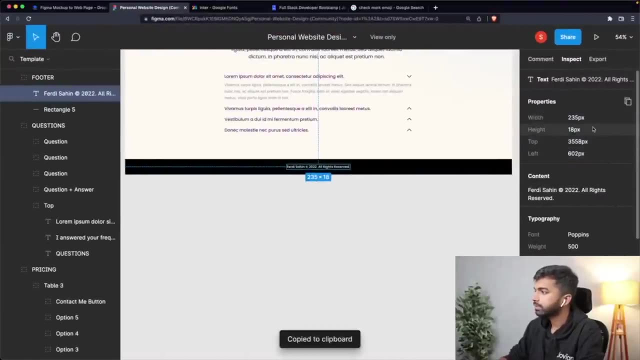 So the color seems to be white. So let's add a color: FF, FF, FF. the color of the pages footer is white. Let's grab the properties, the text properties. So the text properties just seem to be. the typography is just Poppins. 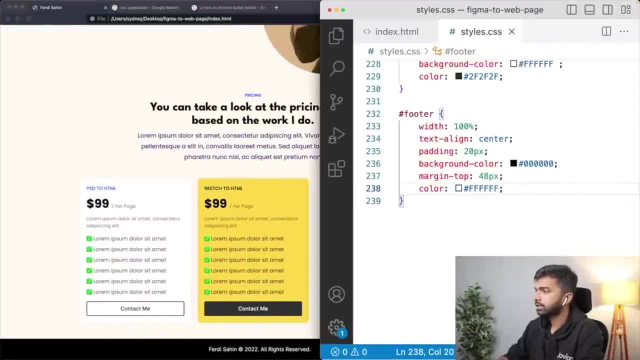 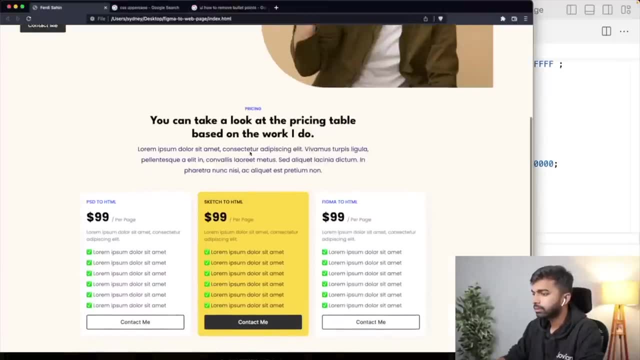 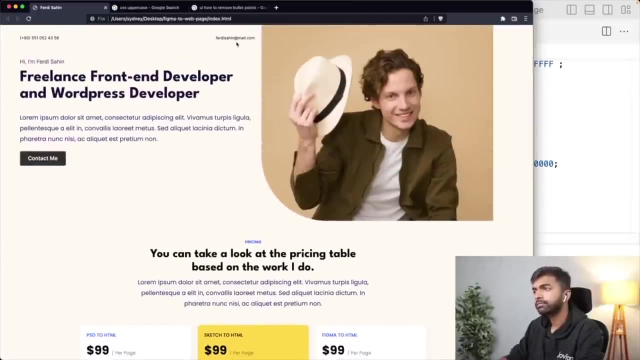 So Poppins: 12 PX, 18 PX. So let me just put that in here as well. Yep, And that's it. So now the footer has been added and the pricing has been added, and we have- I believe you've- achieved- 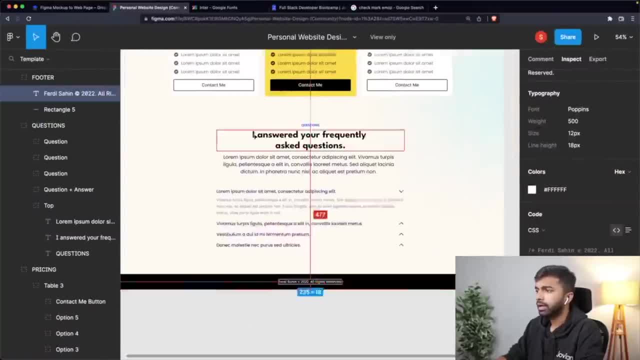 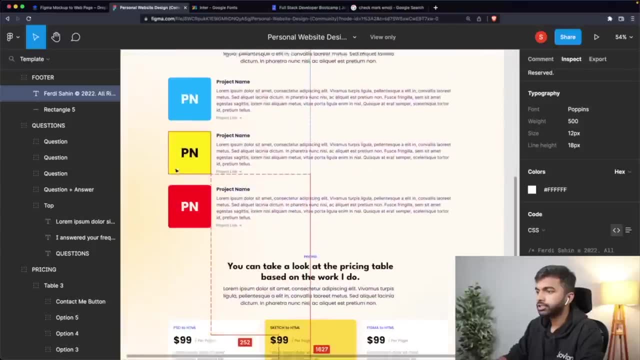 Okay, Yeah, Okay, Okay, Okay, Okay. what we wanted to set, what we set out to achieve, at least in terms of the adding the two sections, The only thing that I'm a little worried about is that this edge seems. 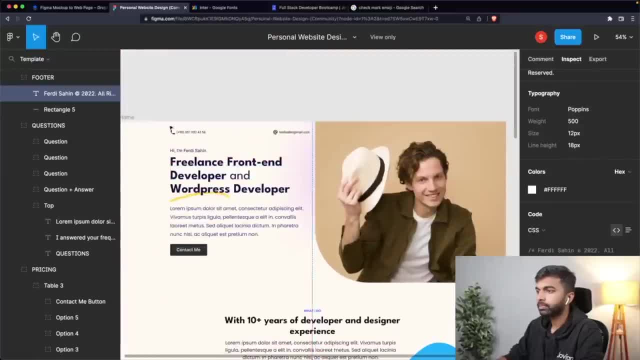 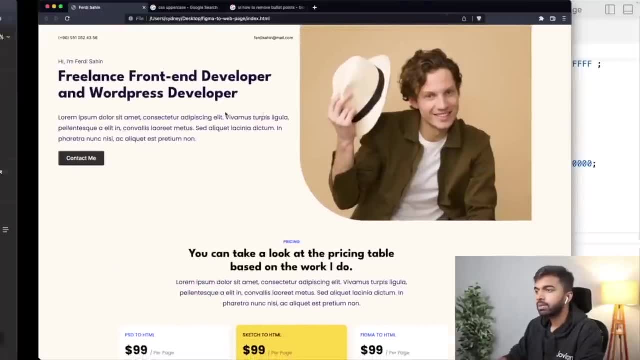 to be lining up with this edge over here right, Which is not happening in our design. Our design is a little more spread out, And so maybe what we might want to do is we might want to restrict the width of this section also to match with this section. Let's see. 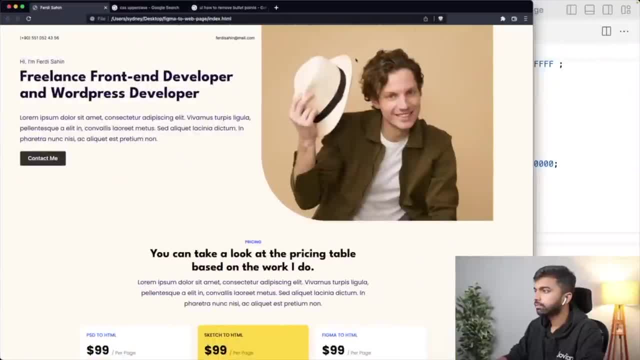 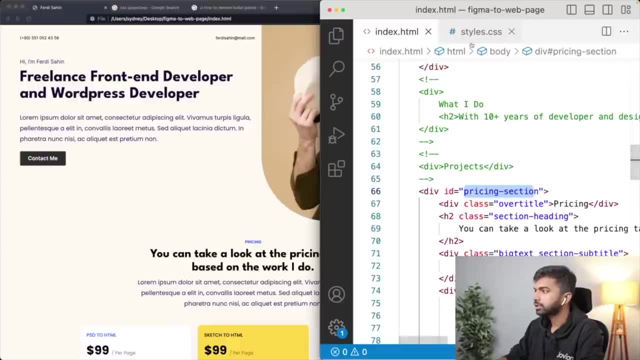 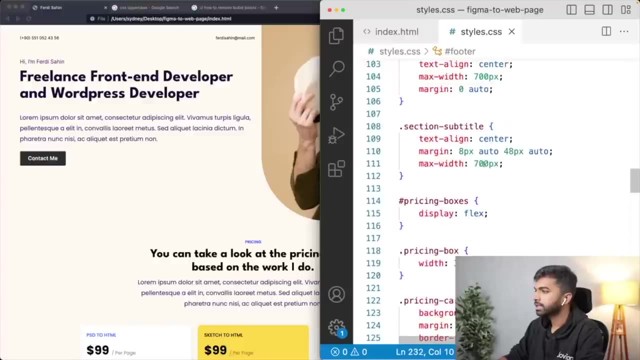 So this is about what is the width of the pricing section. So we have this pricing section and the pricing section, I believe, has a maximum width somewhere set. The pricing section has a maximum width of 700 pixels. No, no, It has a width of 1060 pixels. So maybe let's. 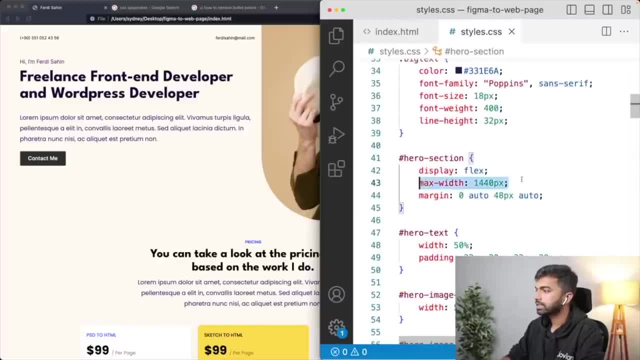 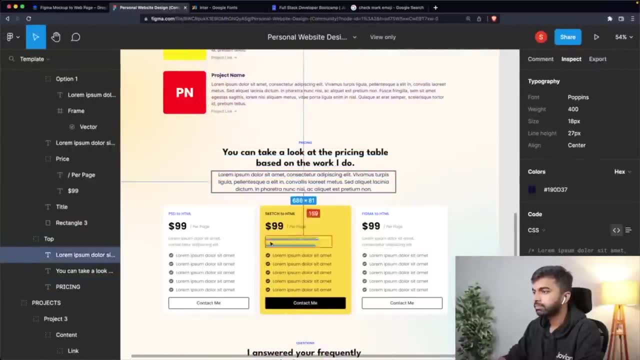 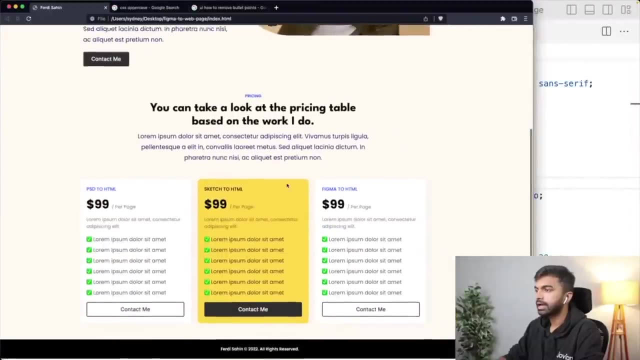 set the same maximum width for the hero section as well. Let's set the maximum width to 1060 pixels. So now everything is centered on the page. You have this pricing section, which is centered, and then above it you have this section, which is also centered like that. Now this: 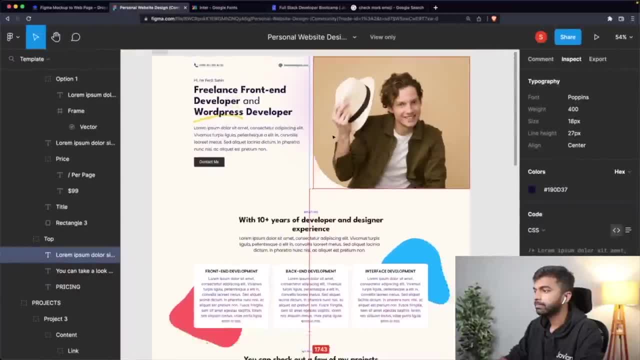 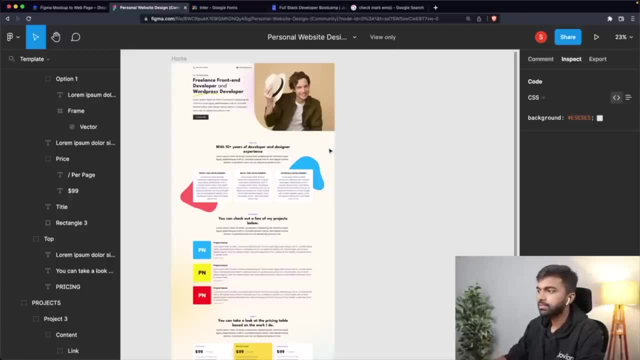 is something that you may want to discuss with the designer. in the design, You see, the image actually sticks out a little bit. but there are two issues with this. If the image sticks out like this, what happens? is that? one, if the content is no longer centered, 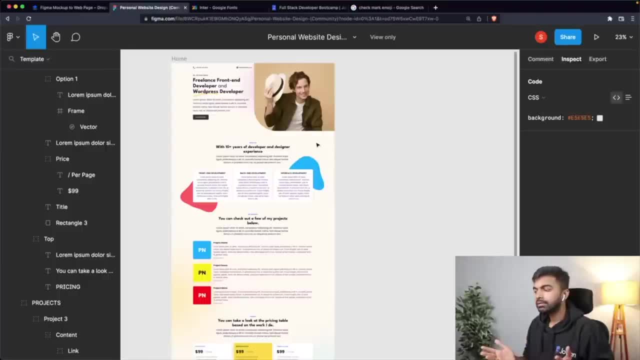 on the page properly? And second, what happens when you have a wider screen? is the screen, is the image still supposed to stick to the side? Probably not right, Because if you have a really wide screen, it's not that you're going to like, let's say, the screen was this wide. from this end, 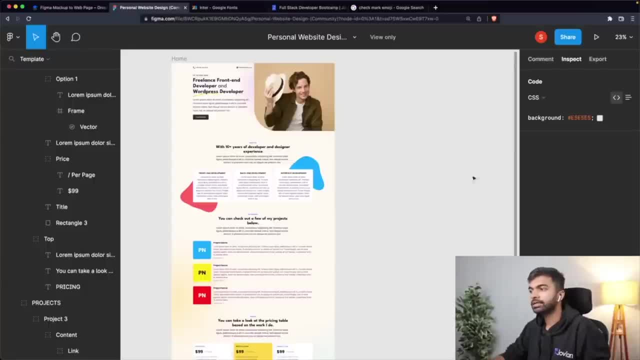 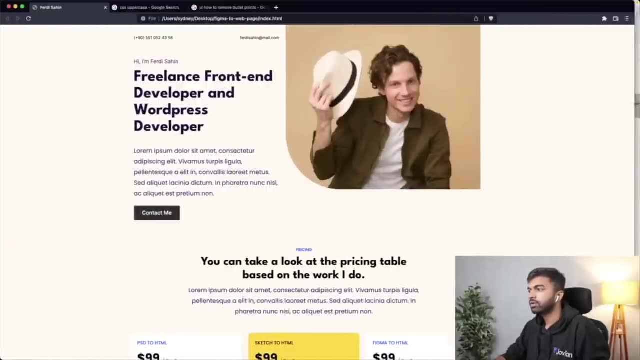 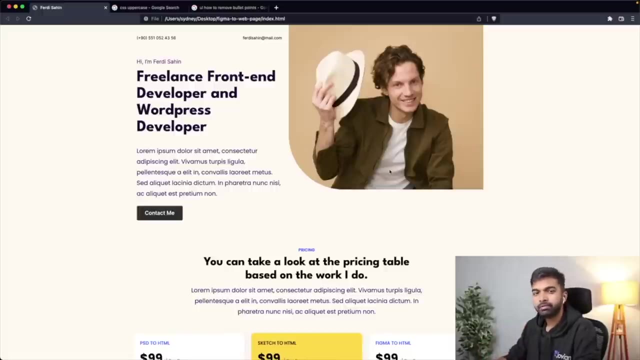 to the send. you wouldn't want the image to just be so big that it sticks out or be somewhere in the corner. Um, so What do we have now? He's like a reasonable- Please Like a reasonable- middle ground to me, But of course it's only the designer who can give the final answer here in. 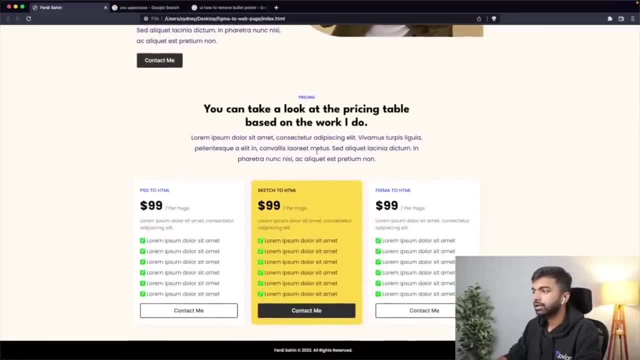 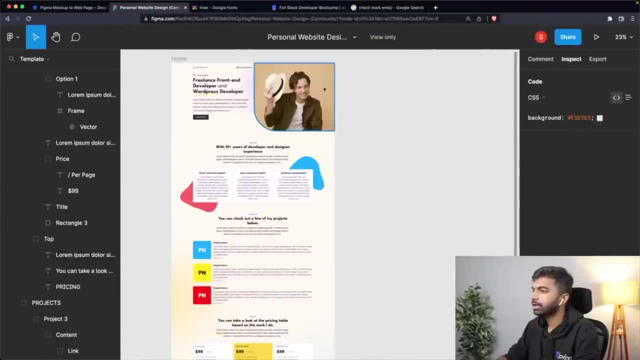 terms of how they want the image to look Right. So this is something that you may want to go back and discuss with the designer. One thing that I will do for this image is I'll probably give it a radius like this on this side as well, just to make it look a little nicer. So it has a radius. 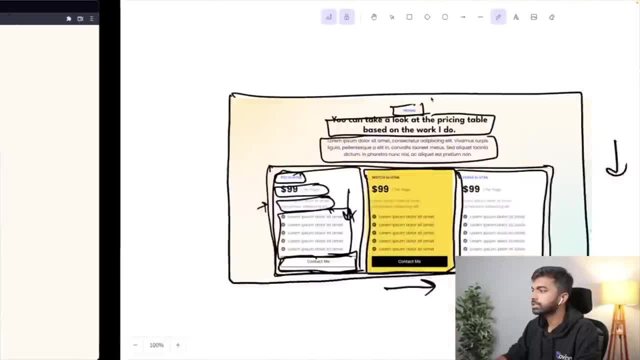 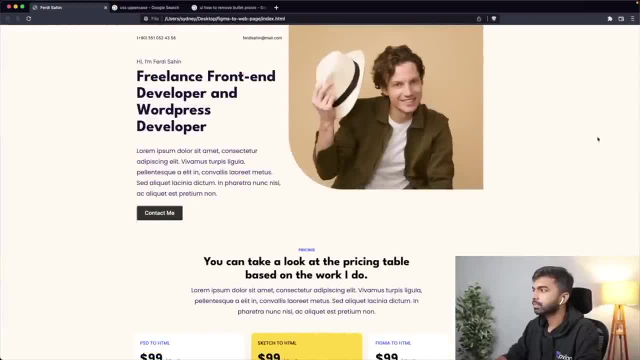 of what it has a radius of about 200.. So let me just go in here And let me add that same radius for the image in my code as well. So I'm going to go to the hero image and I'm going to 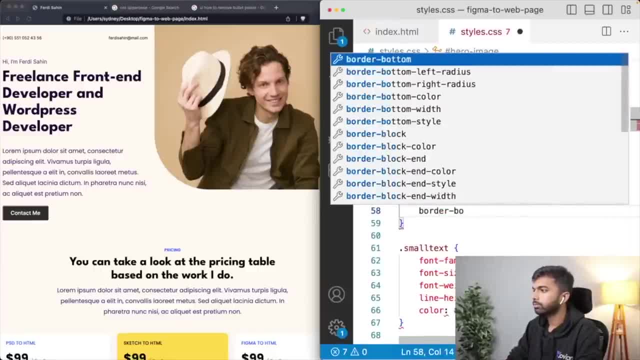 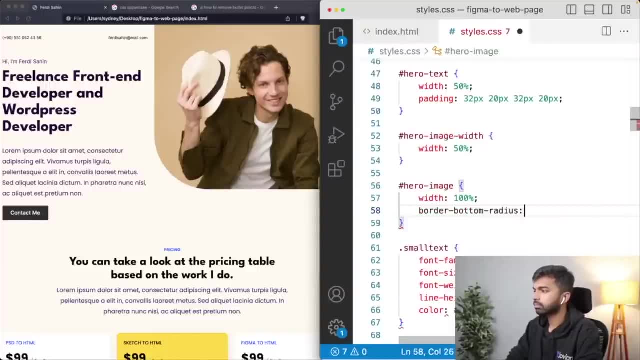 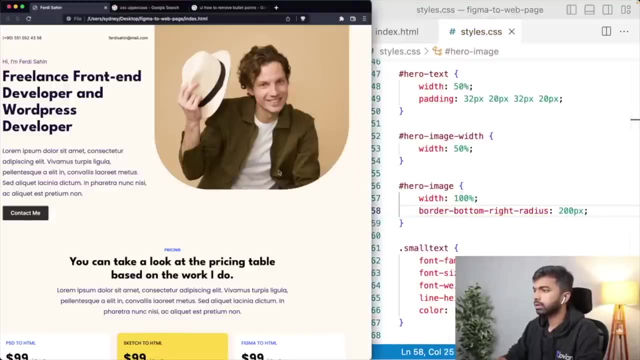 say, border bottom right or border bottom radius, Okay like that. So that's what I'm going to do. So that's what I'm going to do. So that's what I'm going to do. So that's what I'm going to. 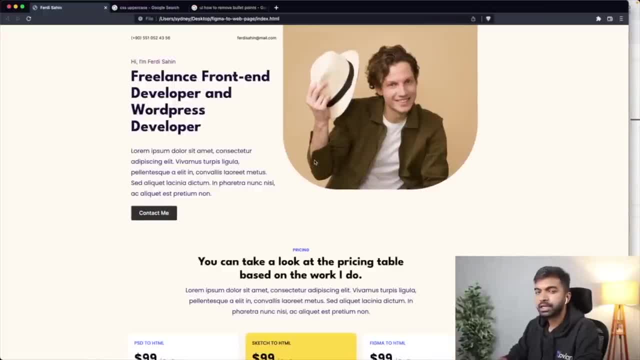 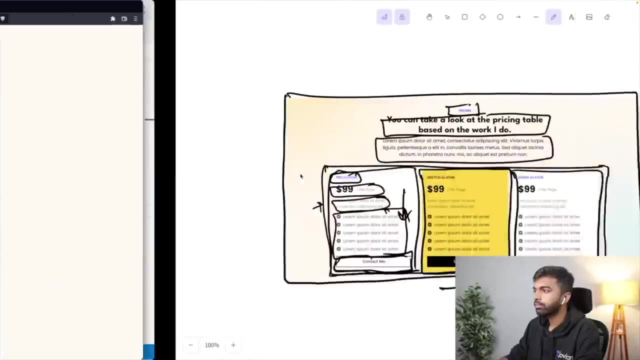 fit And all. the other option is that I expand, I export the image. I don't export it with the radius at all, I just keep it blank. But I think this looks largely looks fine. Of course the content is sticking out a little bit, a little more than I would have hoped. So I may even 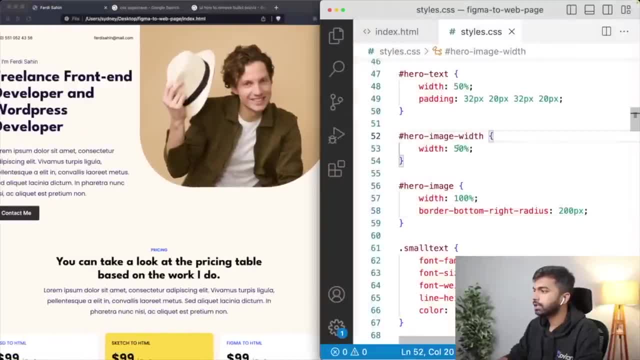 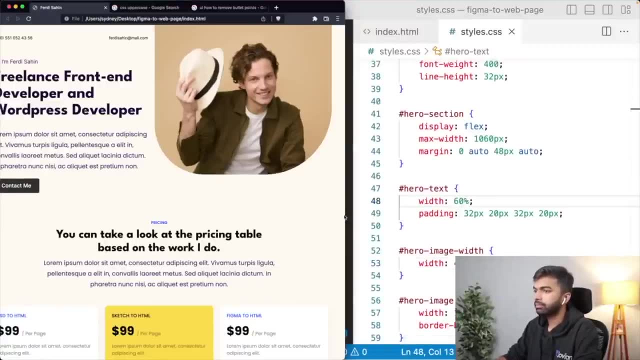 reduce the width of the image slightly. So instead of going 5050, I may go, let's say, 6040 with content and image. Okay, so this is where you may like. when you come to the implementation, often things don't work out exactly as a designer expects, So some things may be need may need to. 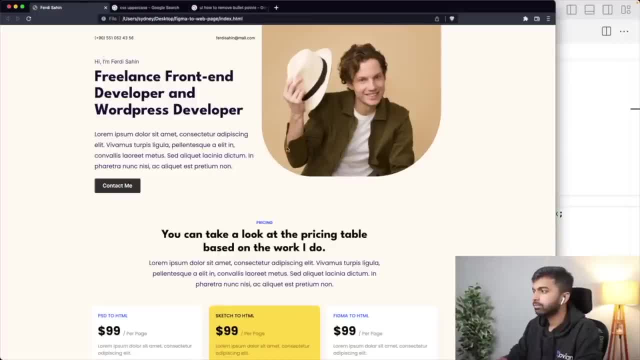 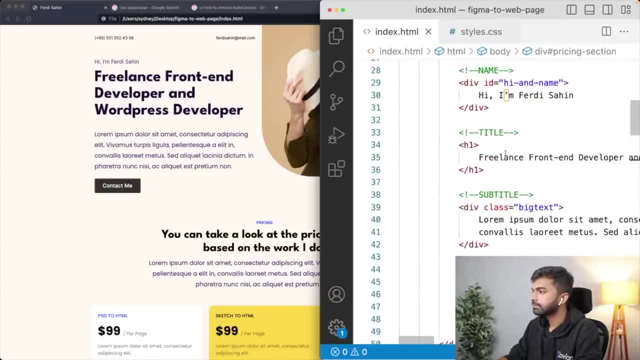 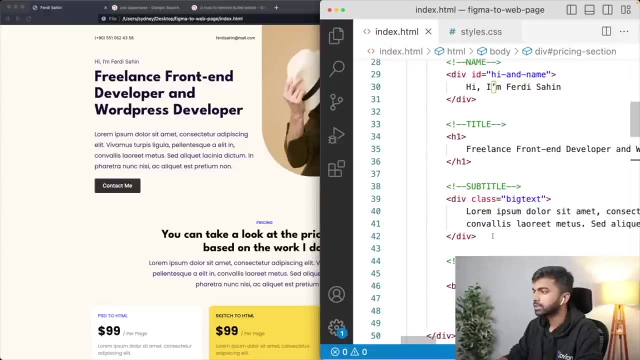 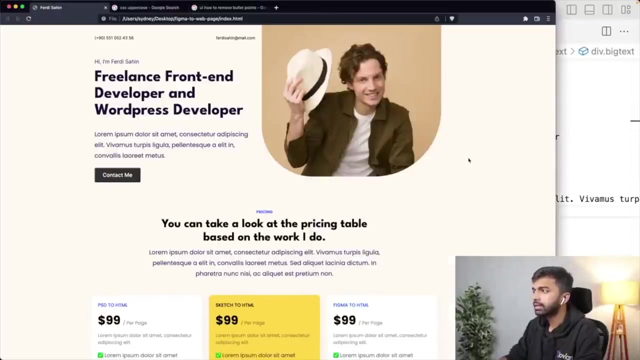 be changed. Might be that we maybe we can reduce like a little bit of the description so that we have one less line in the description. Let's see. So this is the subtitle, And in the subtitle let me get rid of this entire section. Like that. Let me reduce the width of the image. 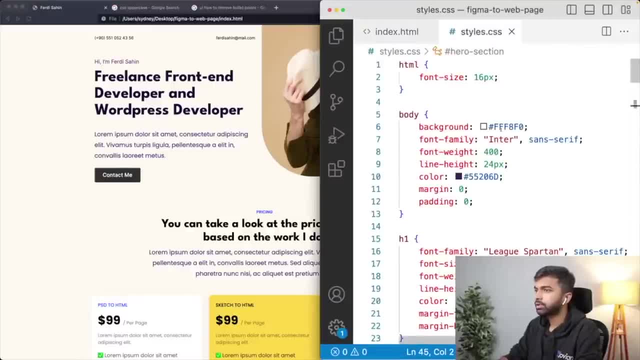 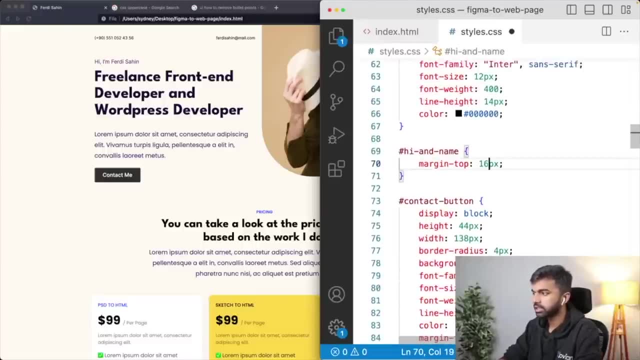 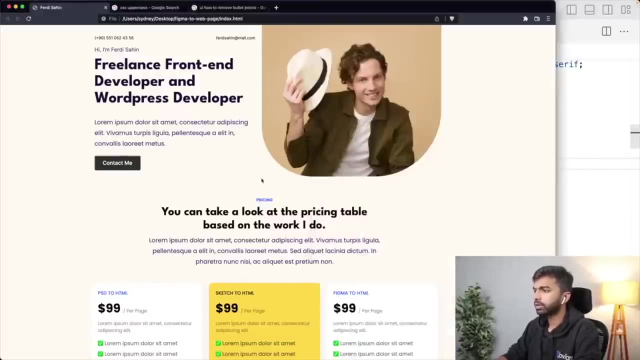 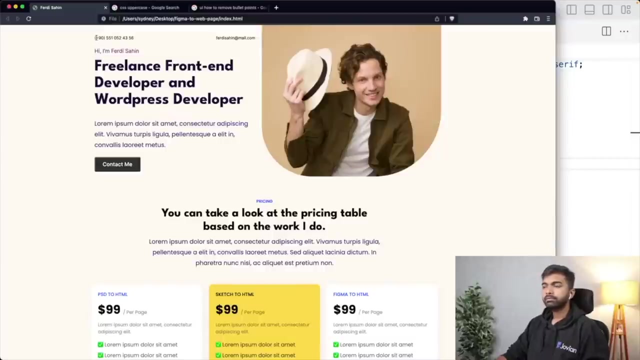 Let me reduce a little bit of the top margin over here. So, before the high M for design, let me- Yeah, let me- just change that to about 16 pixels, let's say, or 20 pixels, Okay, And that looks good. I think this is. this page is looking fairly good. We have this phone. 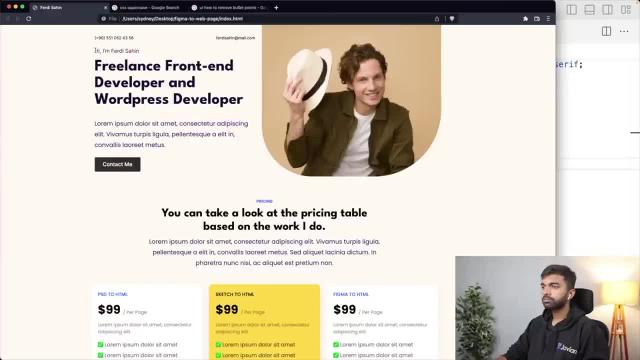 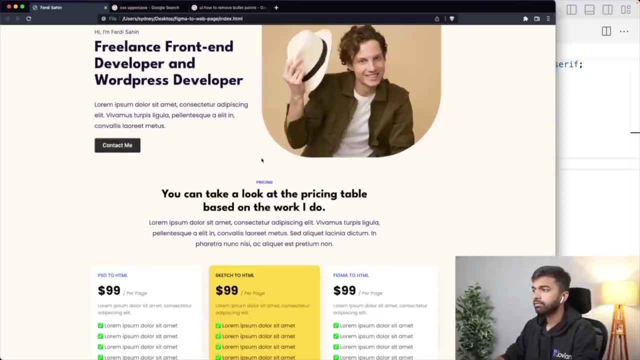 we have this email here, both of this and both of these pieces of information. we have this high freelance front end developer and WordPress developer, a subtitle and a contact me button. then we have this a little bit of a gap. we have pricing. you can take a look at what the pricing 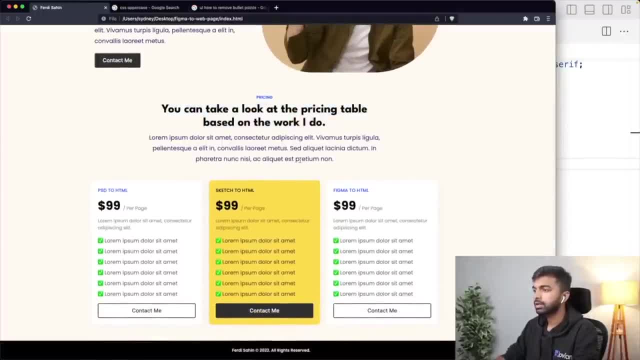 table. at the pricing table based on the work I do, then we have again some description, then we have these three pricing sections, then we have these contact buttons And then finally, at the bottom, we have this for the same: copyright 2022.. All rights reserved. 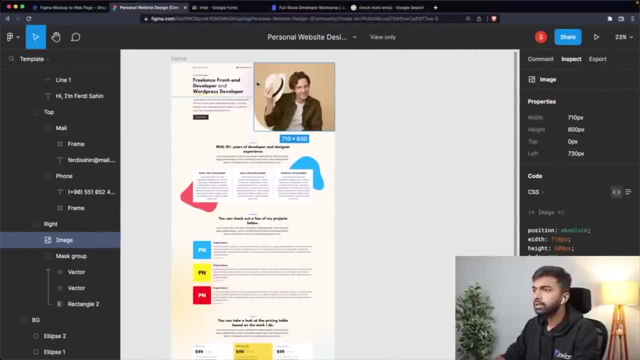 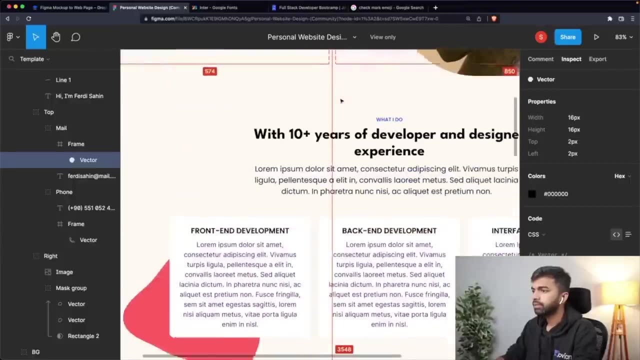 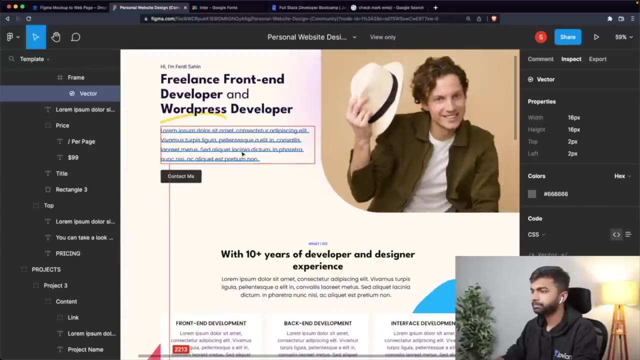 so that's fine too, And maybe the only last thing that we may need to do is add these icons Over here, this icon over here, And maybe also add these icons, these checkmark icons that we have over here. So let's do that, And I think then with that, we'll close for the day. Of course, 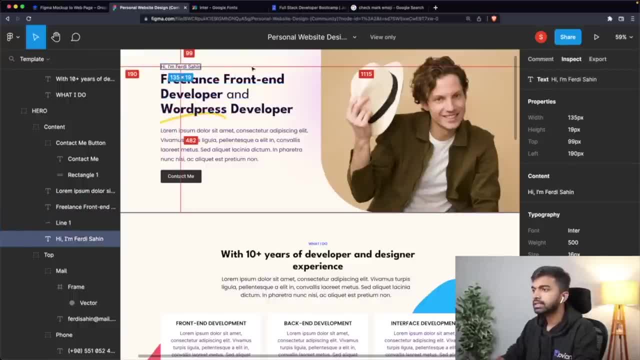 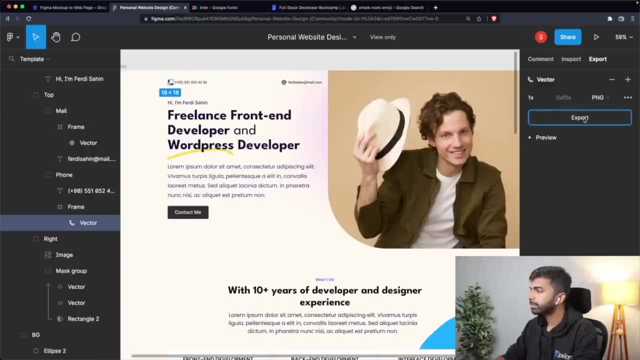 let's see if we can also incorporate this, But I'm just going to add this icon for now. So I am going to export this, So I can go into export And let me export this as a PNG file Or I can also export. 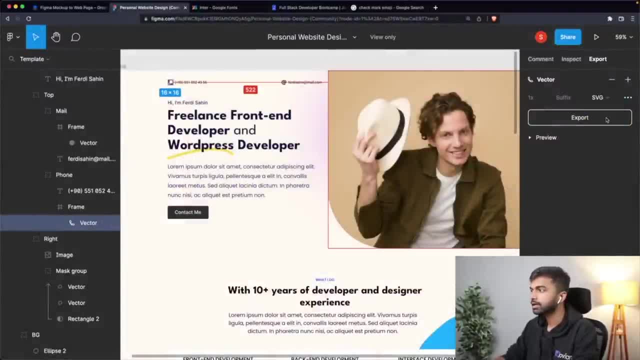 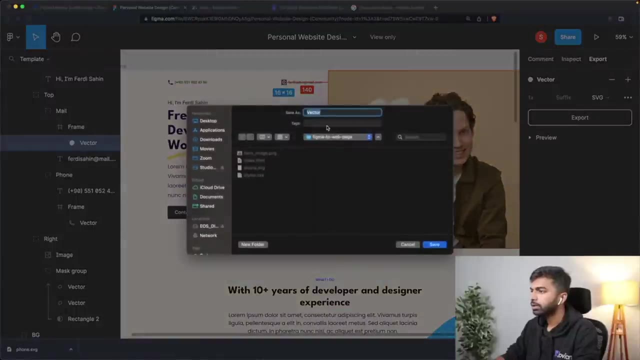 it as an SVG file. SVG is good when you have to resize things, So let me expose, export this as an SVG file, And let me export this as phonesvg or phone. Then let me export this And again, I'm going to export this as an SVG and export as emailsvg And finally I'm 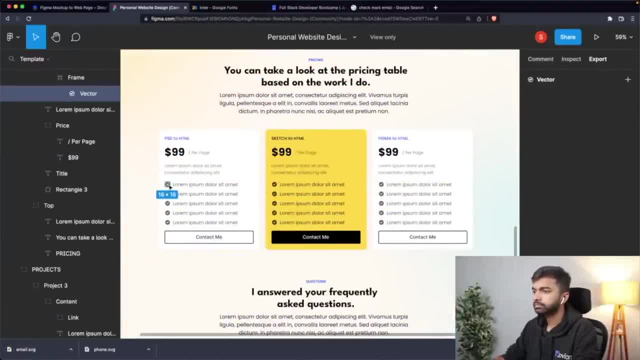 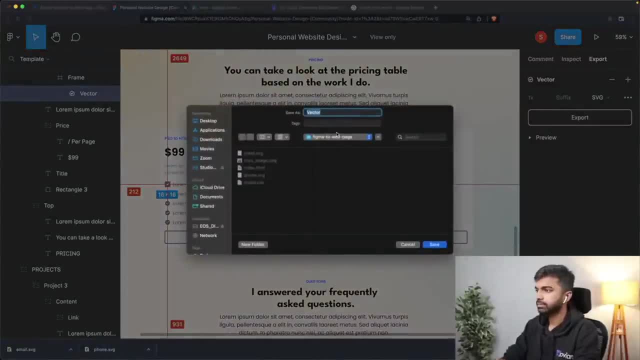 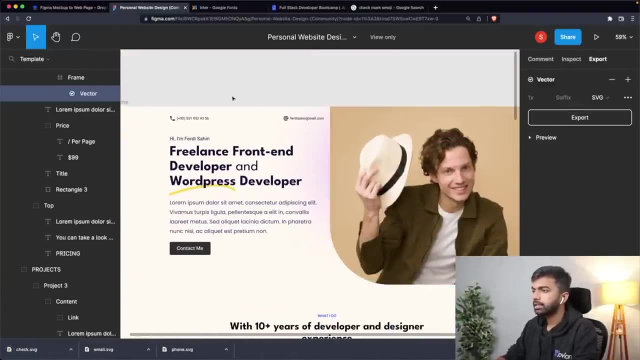 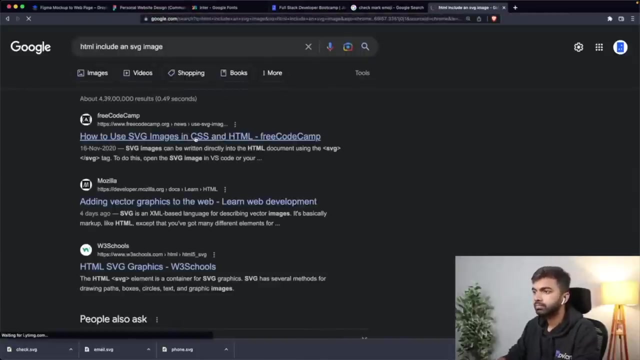 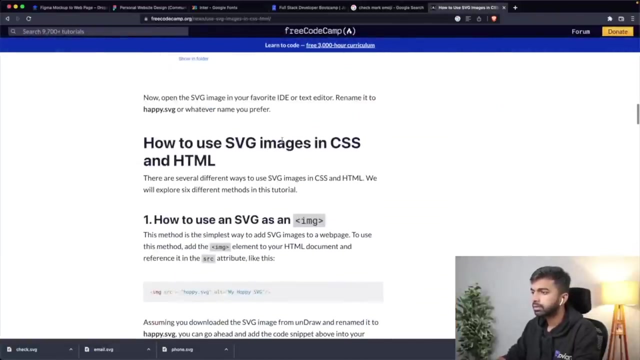 also going to export this checkmark over here, So I'm just going to go ahead and export that again as SVG, as dot SVG. okay, now we just need to incorporate or bring in these SVGs. so let's see HTML: include an SVG image. how to use SVG measures and CSS. well looks. 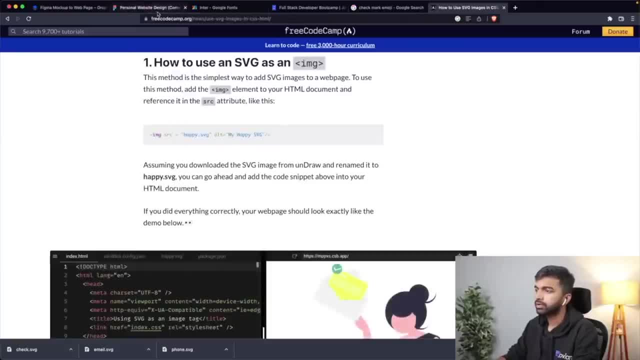 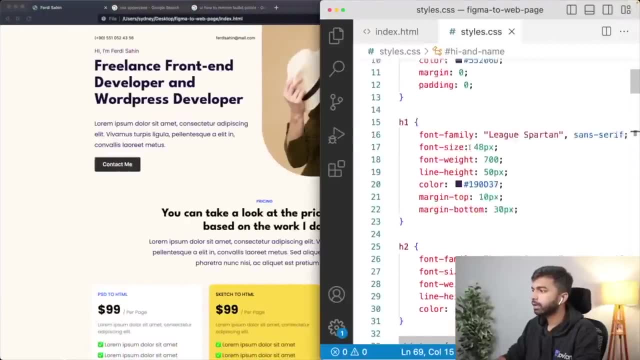 like we can just do this. we can say IMG, SRC, and we should be fine, and we can give it a height and width. so what is the height here? 16 by 16, right? so I'm just going to do that, for I'm going to come in into my text here and I am going 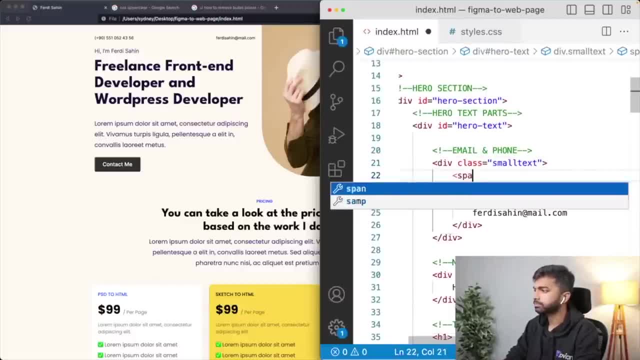 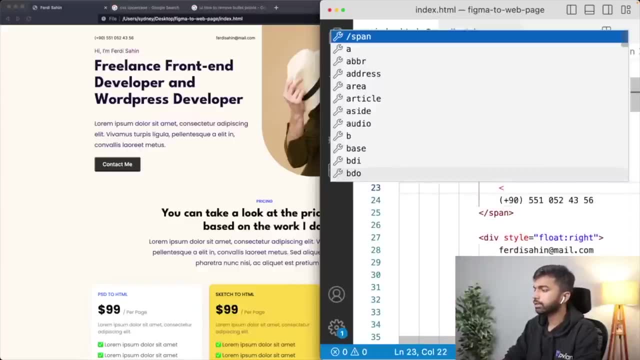 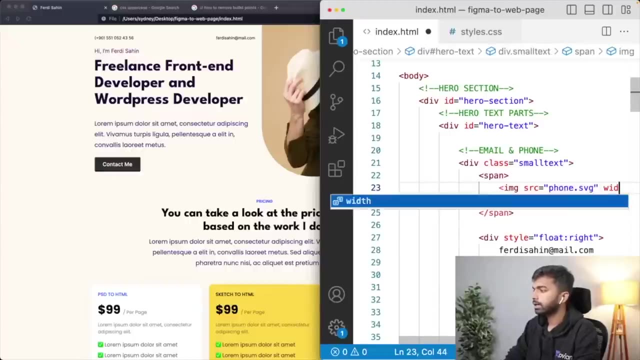 to come in before telephone number. so I'm just going to first create a span so that I have a span around the telephone number, and then I am going to create this IMG: SRC equals phone dot SVG, and let me just set width and height directly here. width equals 16, height equals 16. 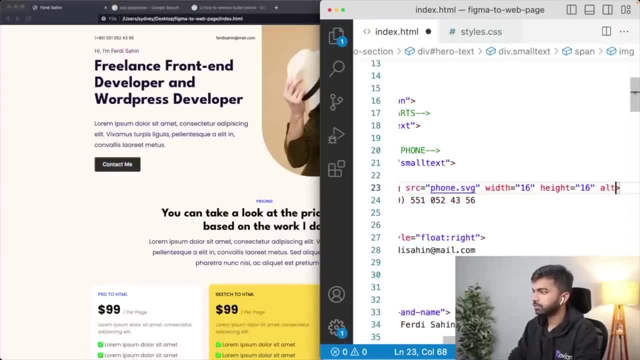 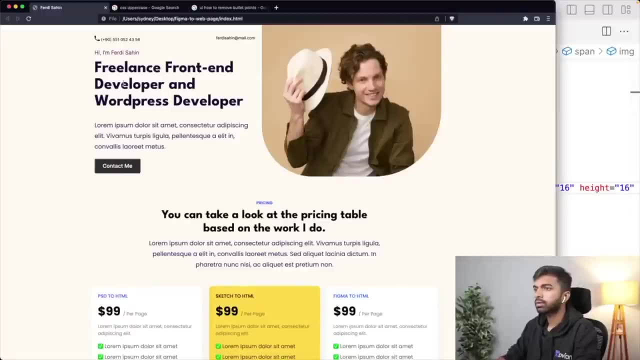 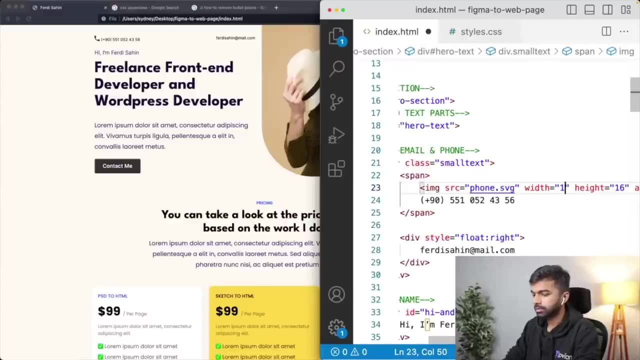 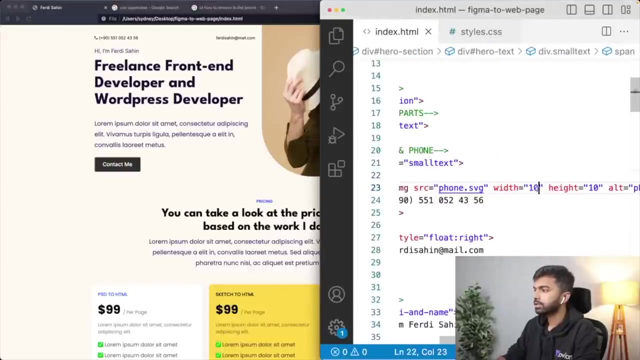 and let's say, alt equals phone. we should always put an alt tag for an image. there you go. it's almost there, more or less, I think it. we probably don't need such a big thing. maybe 10 by 10 might actually do it. yeah, maybe 12 by 12. so that takes. 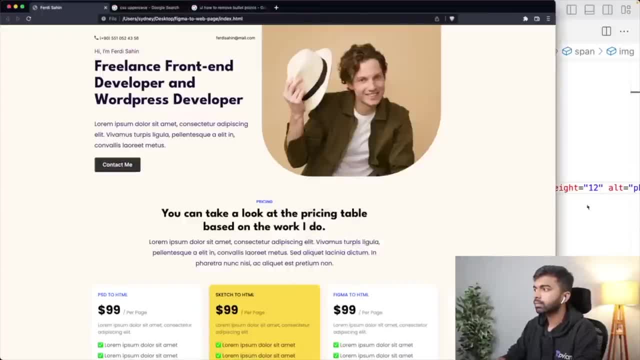 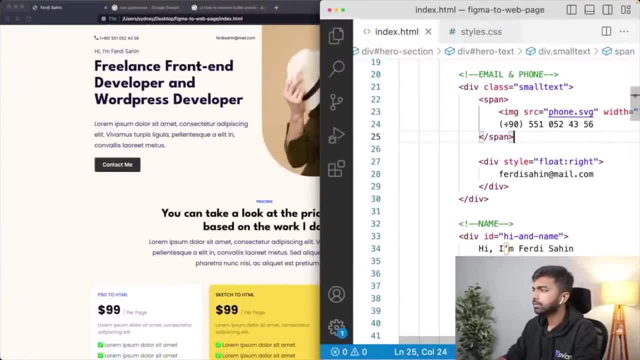 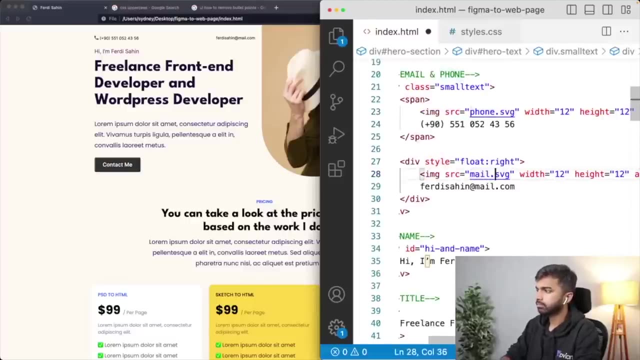 care of that for us. right, let's go ahead and use this. I am putting in something like email dot SVG and reach for it so that I can navigate through this. and yeah, I think that's what it looked like here as well. roughly right, let's get, let's add the email. so 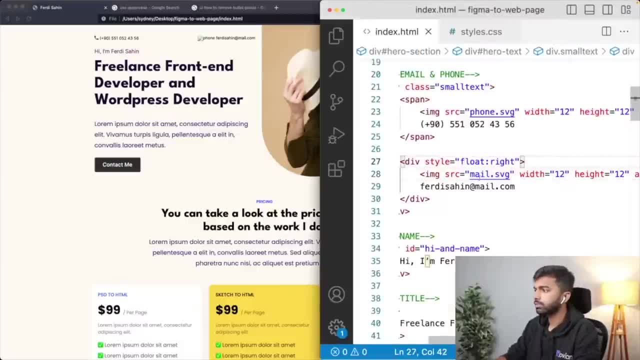 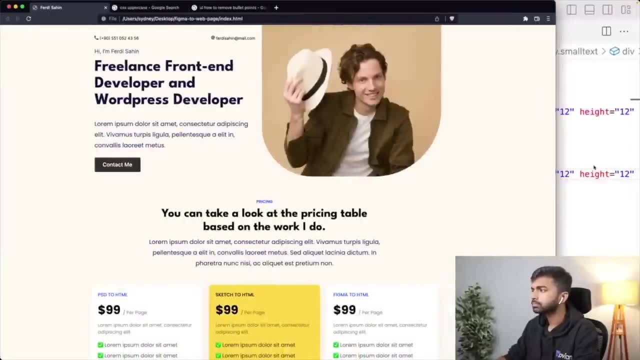 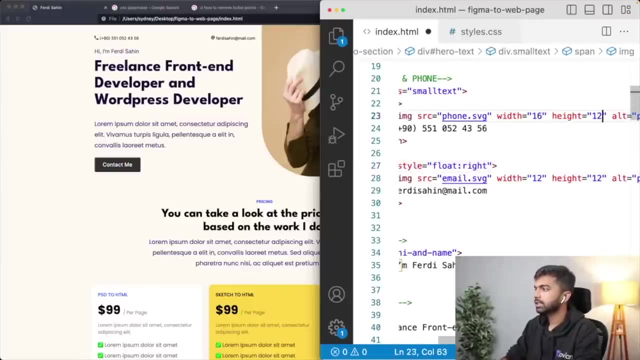 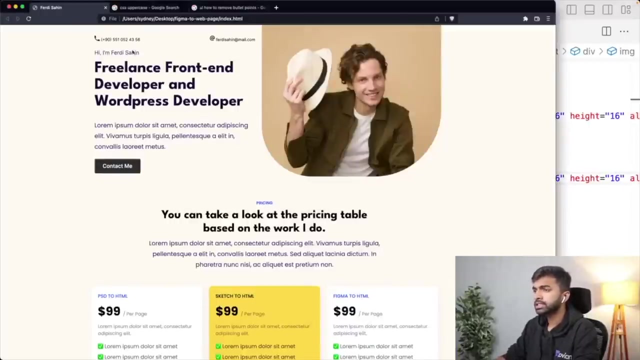 let's again get this IMG here and we'll just change it to mails or SVG, or email nor SVG. yeah, that's roughly what it looks like as well. you could say that this we could just give it like a small margin to adjust, to adjust things a little bit. 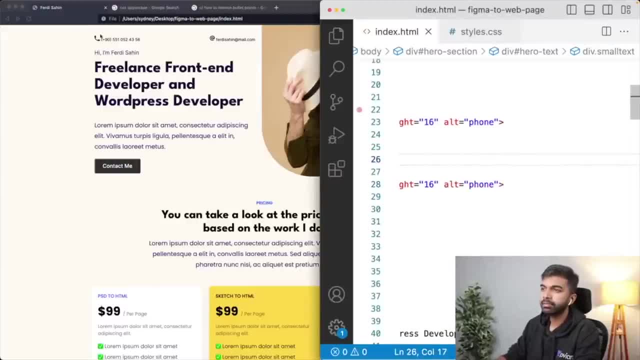 So what we could do is a quick trick. Anytime you want to center an image next to a page, you can. there are more complex ways to do it, but a very quick way to do it: I need to move the image down just a little bit. 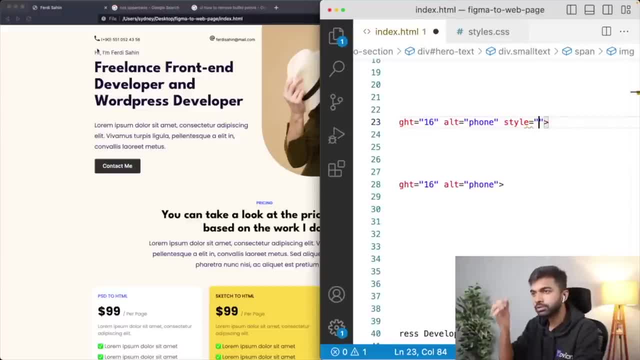 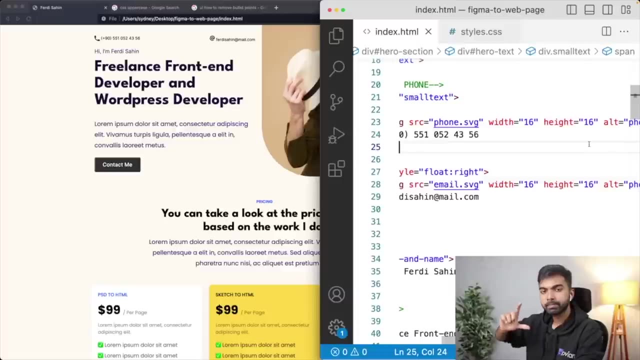 So you want to keep. you want to maintain the rest of the things as they are, but you just want to make move the image down a little bit. You can say: margin bottom minus four PX. Okay, What that does is that does not actually add any additional space. 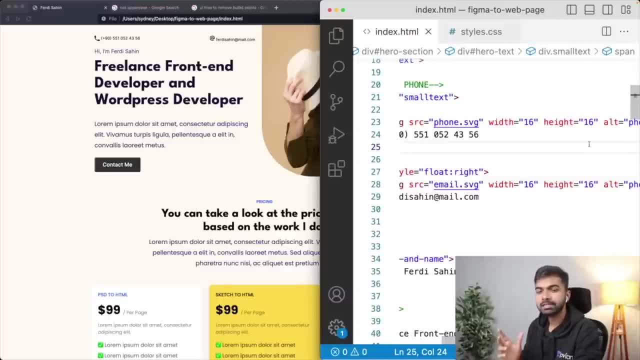 It simply shifts the image up or down. Okay, So negative margin is a very interesting thing that it does not add additional space. It simply shifts the image left or right or up or down, as you say, And similarly I'm also going to add a margin bottom minus four PX over here. 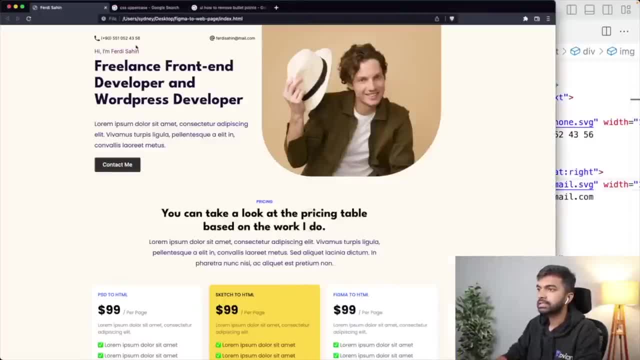 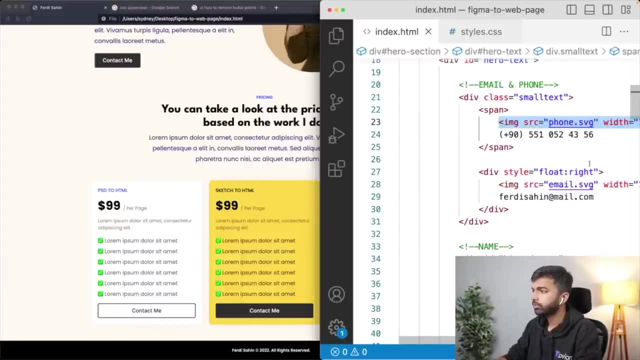 So play with negative margins. But now you can see that These things are all nicely lined up and let's go in and add all of this here as well. So I'm just going to copy this IMG and I'm going to put it in the place of this tick. 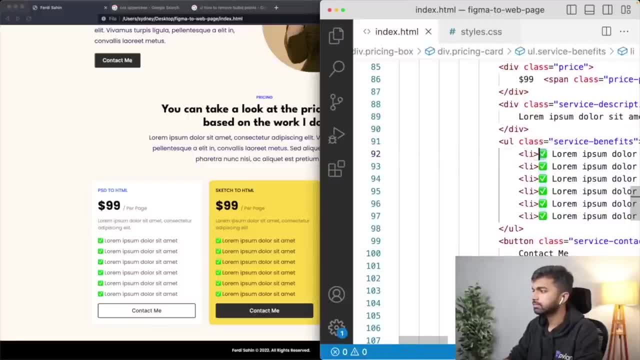 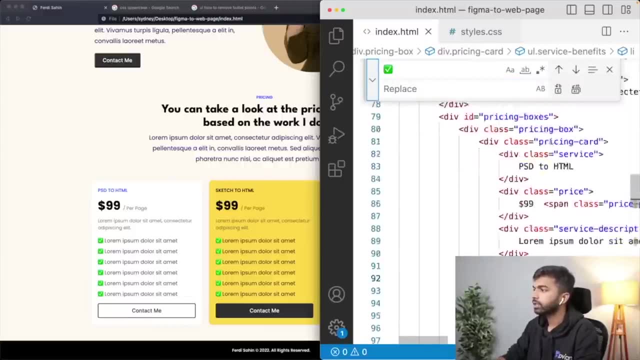 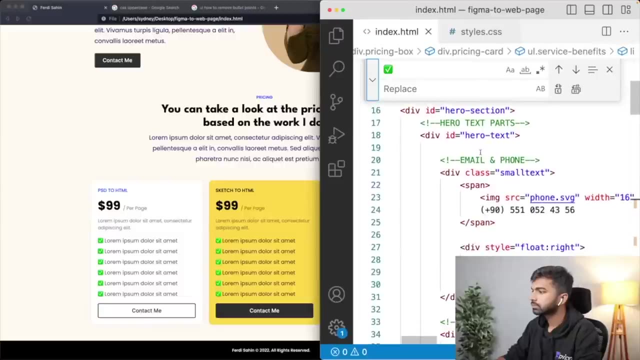 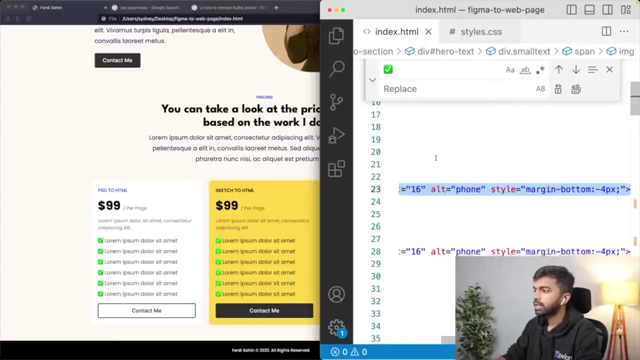 mark over here. So I'm simply going to replace. well, let's do this, let's go find replace. So I want to replace the tick mark with this IMG tag over here. Okay, Let's first replace one, then we'll see if that is what we want to do. for the rest, as 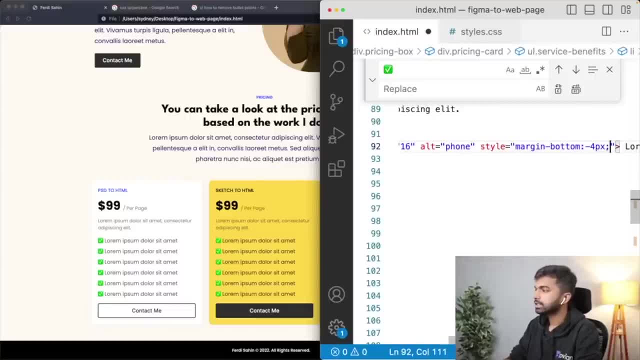 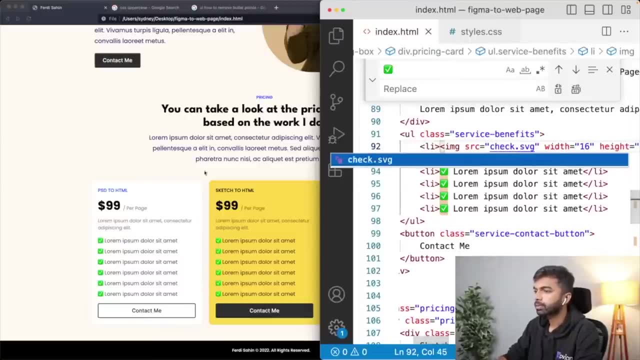 well, Right, So let's put that in here. Let's get rid of this margin bottom. I think we may not need it- And let us just put checksvg and let's reload the page. Okay, I think we may need a slight bottom margin to adjust it. 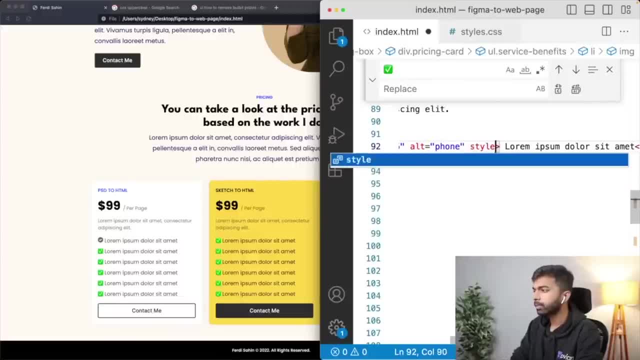 Okay So whenever you have icons next to text, Okay So margin bottom is your friend. So margin bottom and negative margin bottom, in most cases minus 2px. Let's check that. Yeah, that looks fine, So now let's grab that. 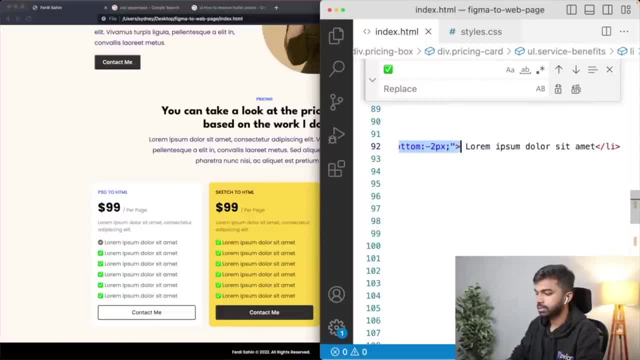 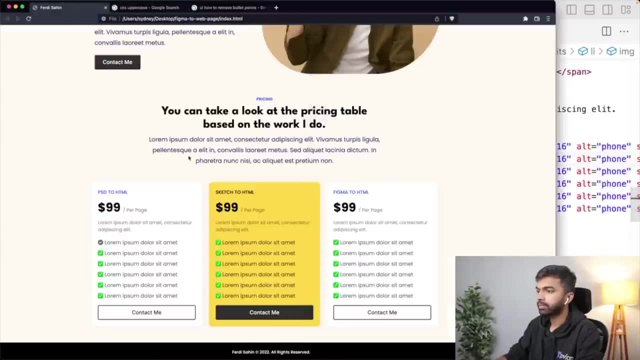 And let's say that wherever we have this tick symbol or this tick emoji, I'm just going to replace them all with that, Okay, And I've replaced everything, And now you can see that my tick symbol is showing up as expected, Okay. 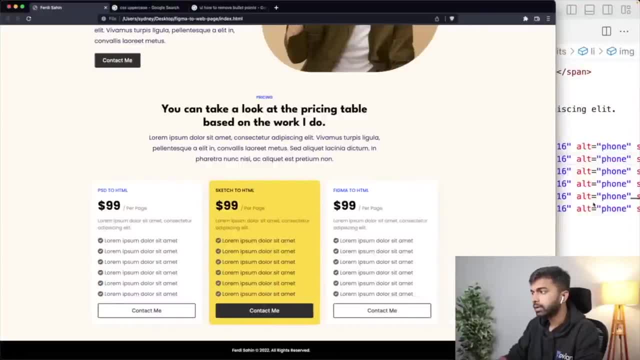 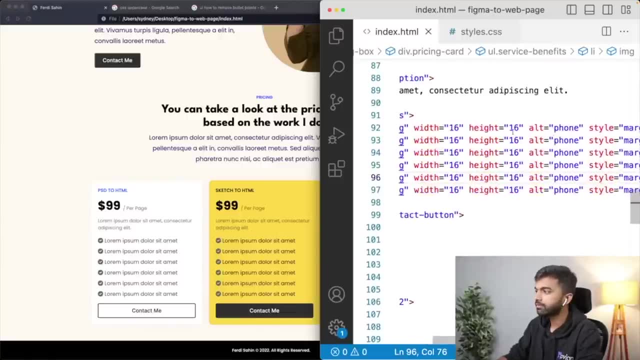 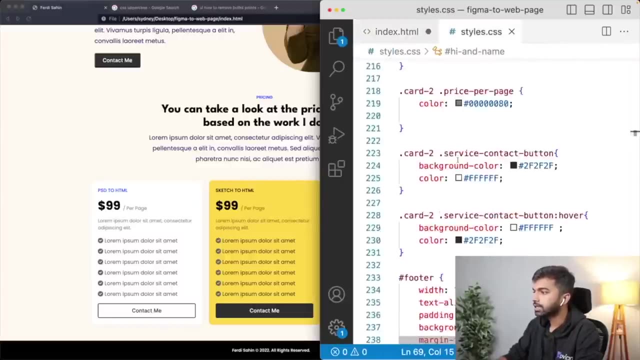 Yep, I could even just if I wanted to make sure that these width, height and et cetera, and style margin bottom. if I don't want to repeat this everywhere, maybe another thing that I can do is, instead of just repeating it like that, I can just create a class called dot. 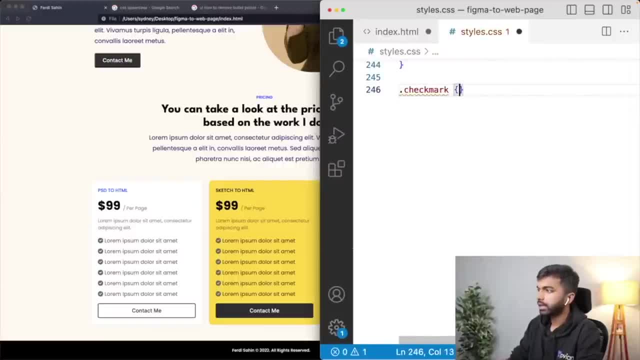 check mark And for dot check mark, I can say that I want margin, I want width to be 16px. Okay, So, Is that 16?? Yeah, 16.. I want height to be 16px and I want the margin bottom to be minus 2px. 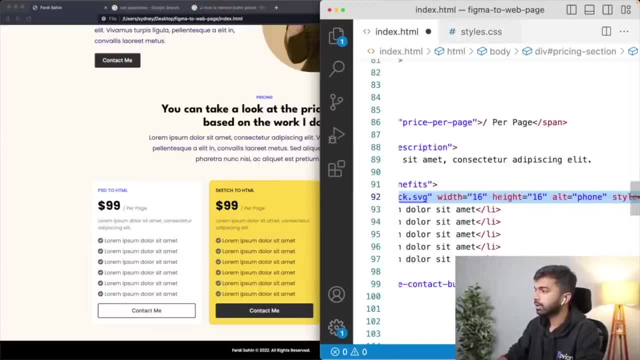 And now I don't actually need to do this. I can. oh, the alt tag is also wrong. We don't probably don't need an alt tag here. I could just give it a class Okay. Class equals check mark Okay. 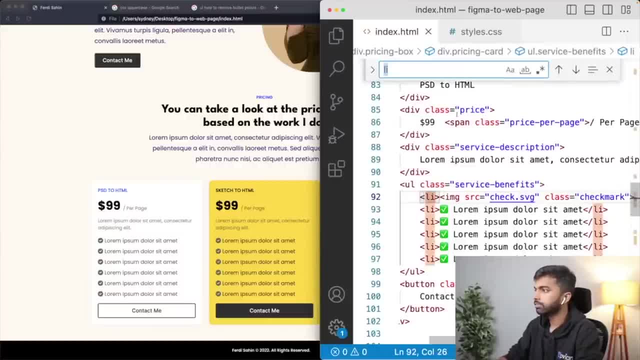 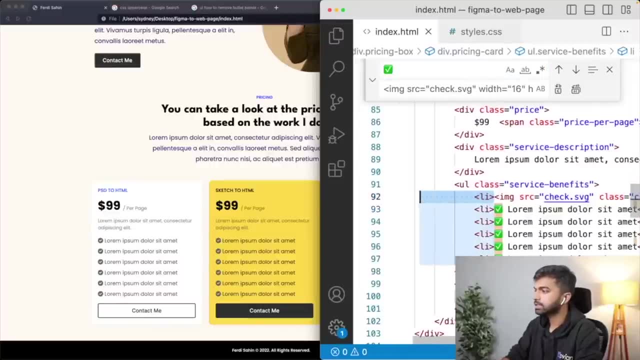 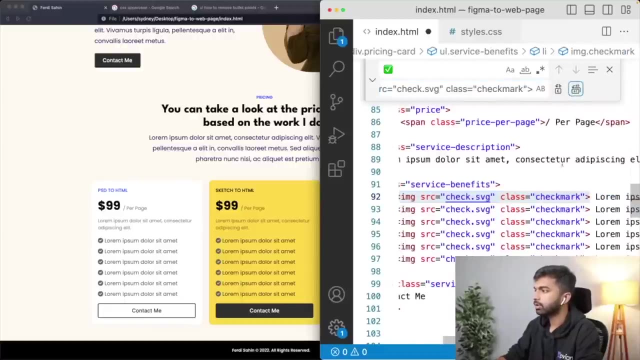 And I can replace this, So I can now go back into the find and replace, And what I want to replace is this: And what I want to replace it with is this: img, src and class equals check mark. And let's replace them all. 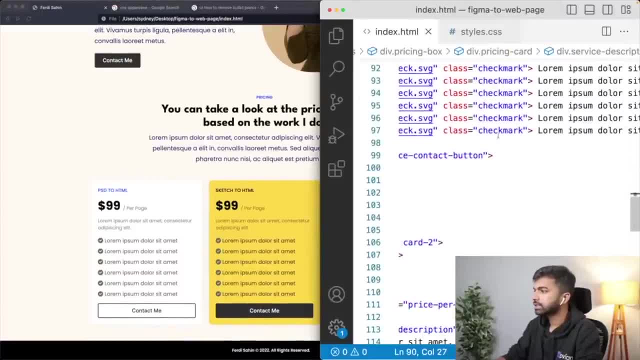 And we get exactly the same result, right With, of course, this time we're using class, We are not repeating a bunch of stuff. Okay, So in case we need to change the height of the check mark or something, let's say we: 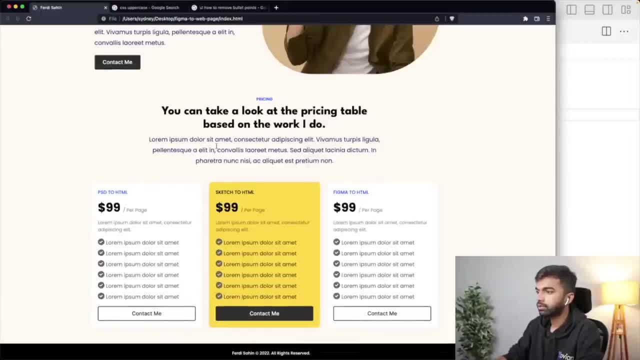 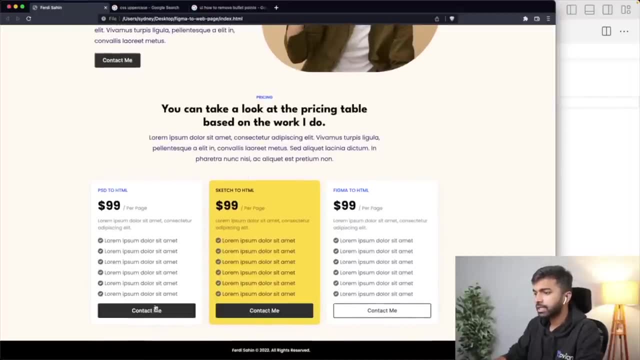 want to change this to 20.. We can do that very easily, Not that we have to. I think it looks fine, Okay, So I think this is a good place for us to stop. We have replicated the hero section closely enough. 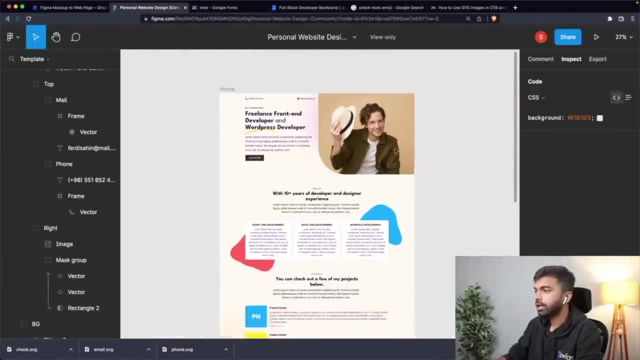 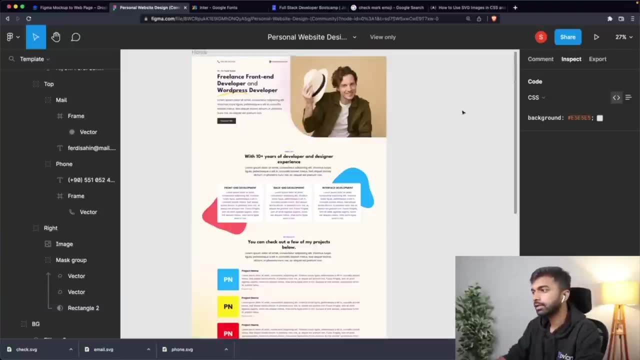 I personally did not agree with the design decision to extend the image outside of the center because that creates problems in centering the content, But I think it's a good place for us to stop. I think it's a pretty good place to stop, because that creates problems for us to extend the. 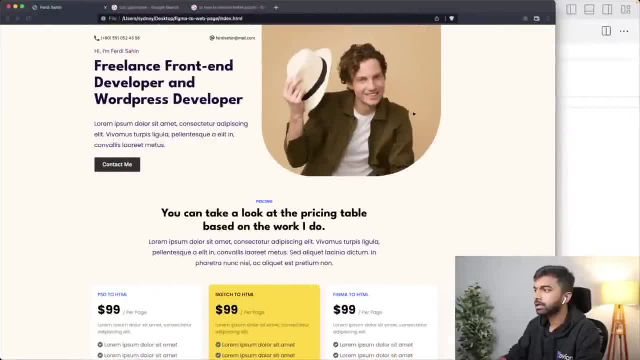 content. I think it's a good place for us to stop So it doesn't end up looking that way, because it's going to create problems for us to extend the content visually, And that also creates problems with larger screens. So instead of what I went with is I simply centered the image. 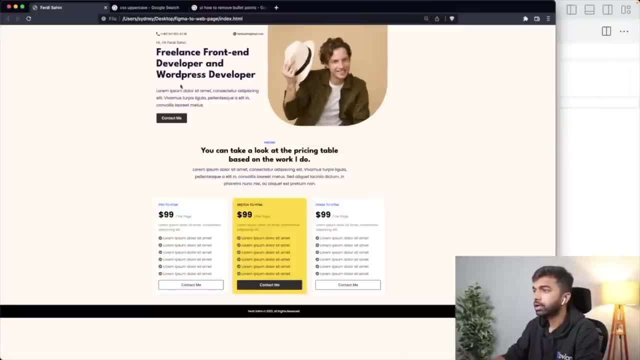 I simply centered the image or the entire content of the page here And I have gone ahead and I've added this heading and, of course, reduced the sizes a little bit so that things probably fit in vertically. then we added the pricing section. You can take a look at the pricing table and in the pricing table. 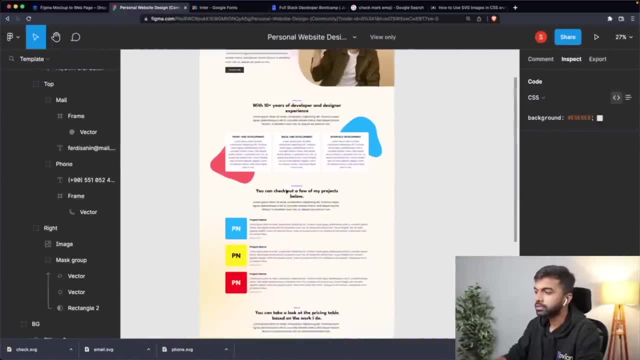 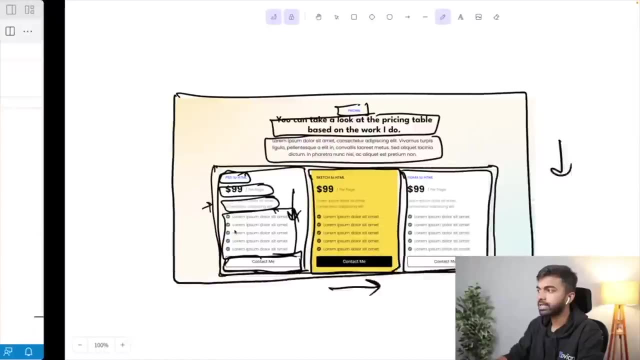 We added all the specific sections. So I'm sure when you looked at it, the design may have seemed fairly complex. but as we just start approaching it step by step, as we break things down, identify. okay, what are the boxes looking? 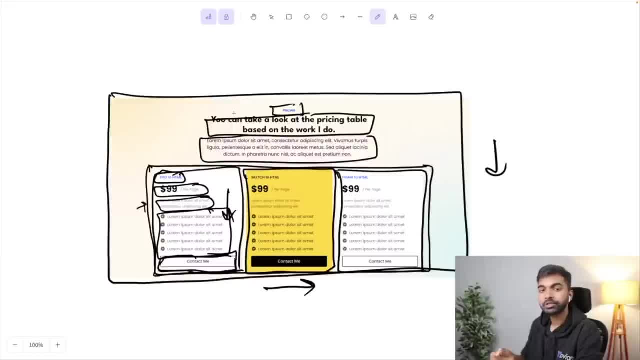 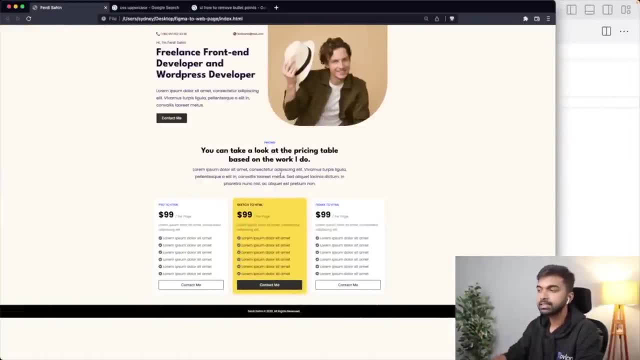 like, and are the boxes arranged in a vertical direction or a horizontal direction? things become a lot easier And then you just have to go element by element, make sure it has the right styles and you can achieve any design, no matter how difficult it looks. And of course there are. 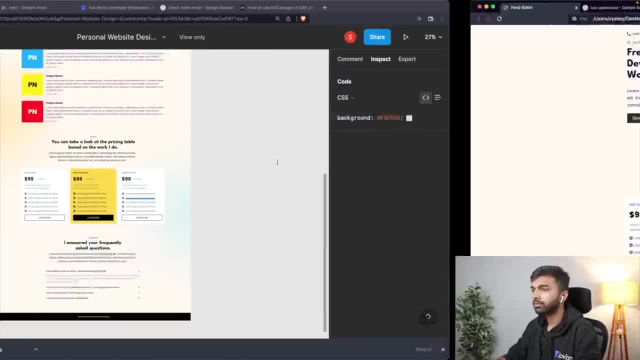 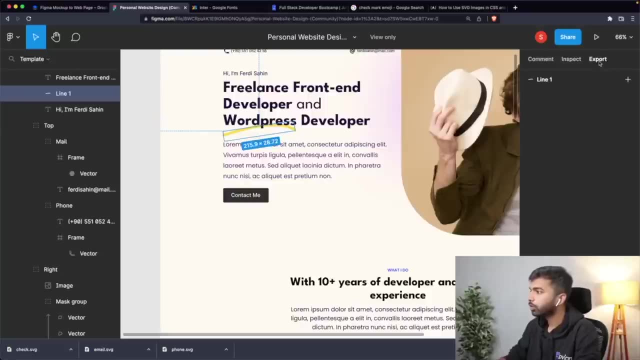 cases where you need, like, custom shadows. you may need to overlap things on one another, Like, let's say, we wanted to do this, How exactly would we do that? Well, let's grab it, Let's maybe export it, Let's see what we can do with it. Let me again export this as an SVG file and in an 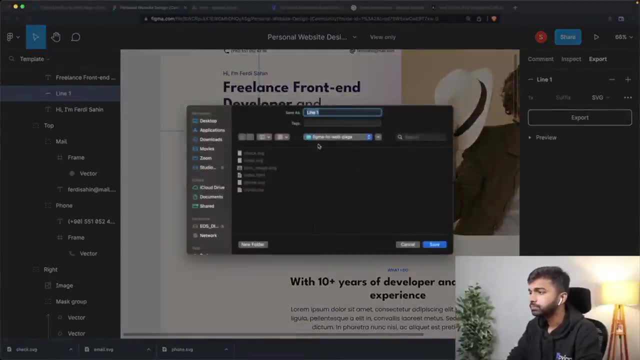 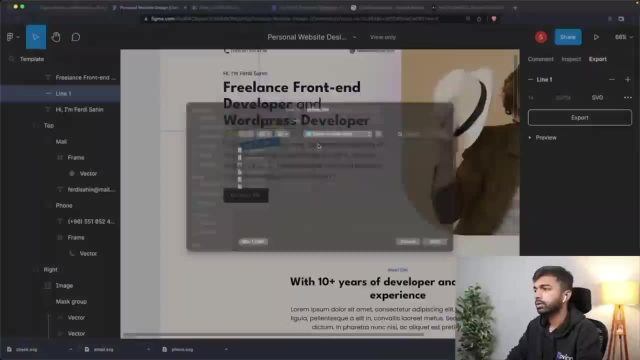 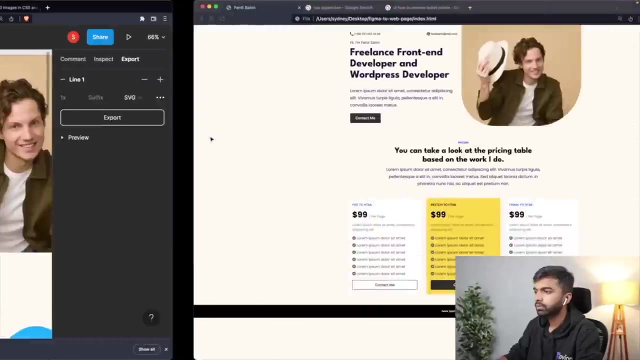 SVG file. let me just export it to line below, or let me just call it yellow line, And let's see how exactly we can fit this. So we want this to show up right below the H2,, right? So let me just show that right below the H1.. 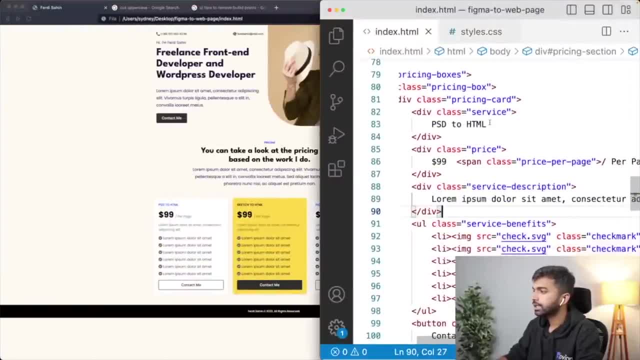 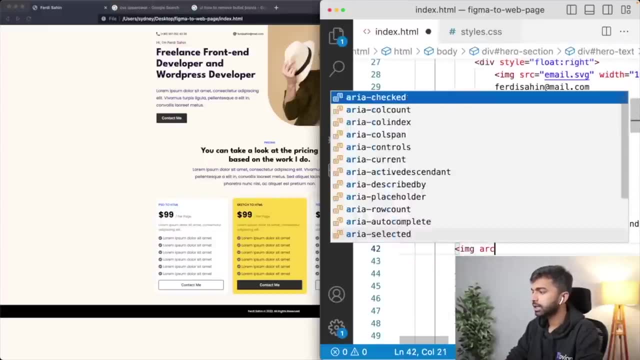 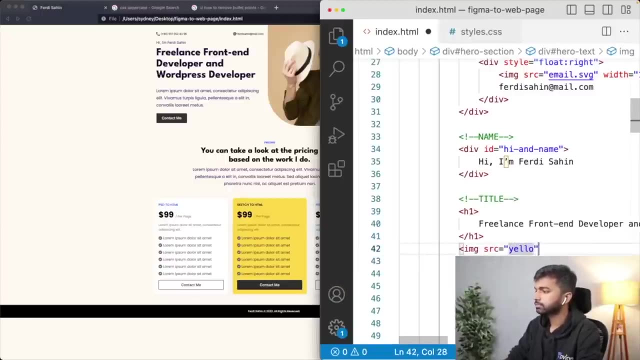 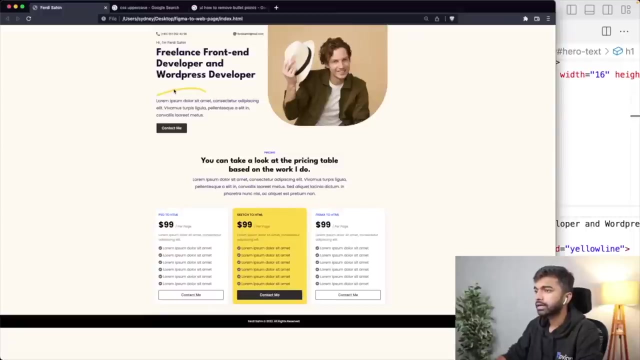 So I'm just going to come in here and I am going to say, below the H1, I'm going to add this image: img src equals yellow linesvg And I am going to say: just going to give it the ID yellow line, Okay. So here's what that looks like right now And again: 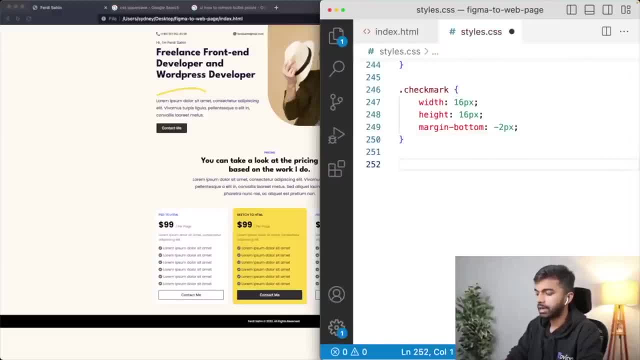 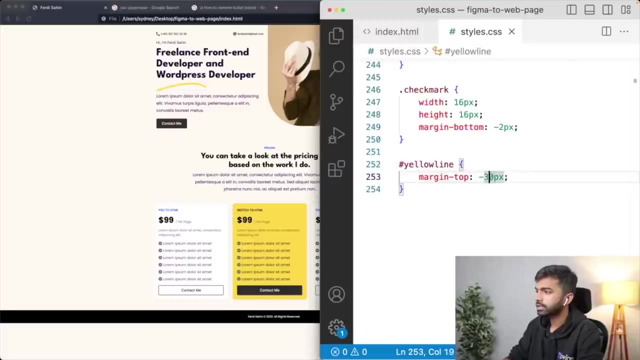 I can use my margin trick. So, um hash yellow line, I can say margin top this time, and I can add a negative top margin minus 30 PX. Let's see what that does. Yup, That's getting us close. minus 40 PX. Nope, Doesn't do it. Minus 50 PX. Okay, Maybe I can. 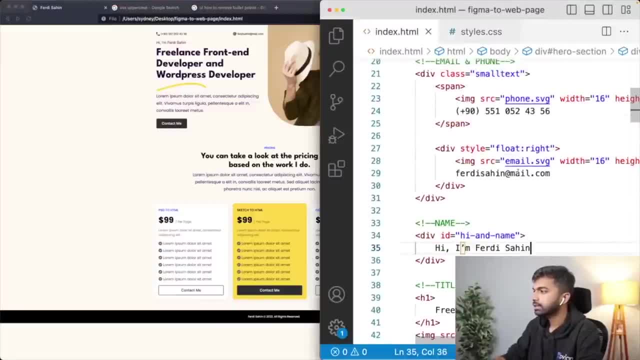 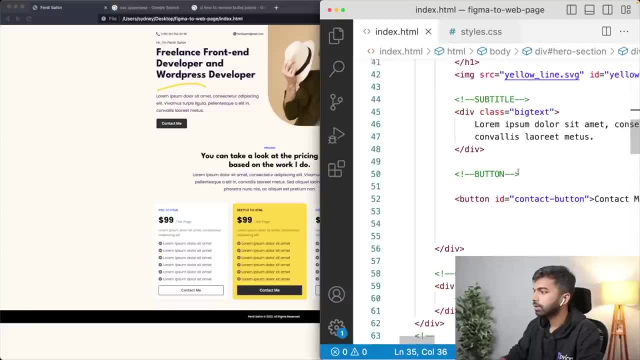 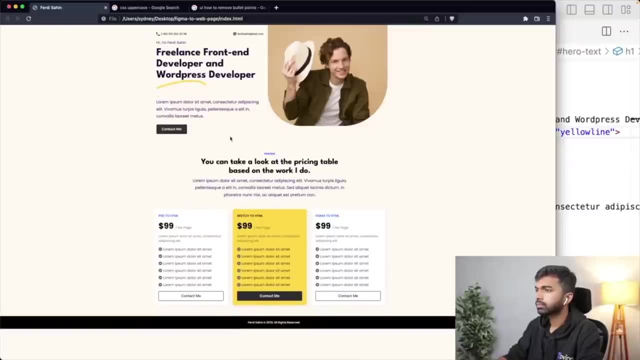 put this yellow line inside the H1 tag, because the H1 tag has its own margin which I cannot get rid of. So let's come back here. Let's take that yellow line, Yeah, And let me put that inside. Yeah, that is better. 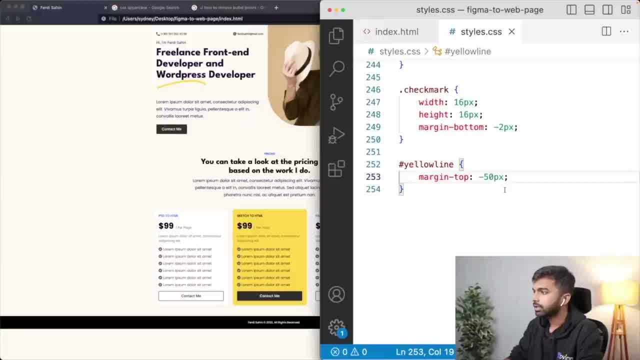 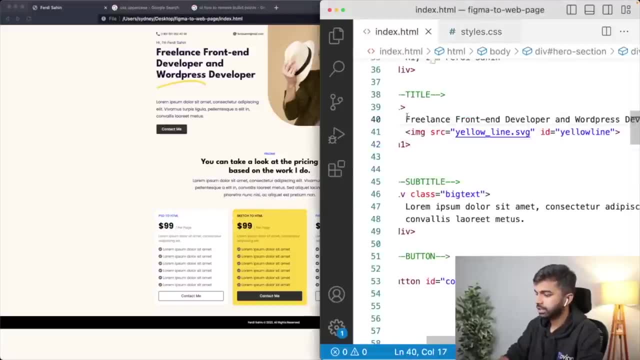 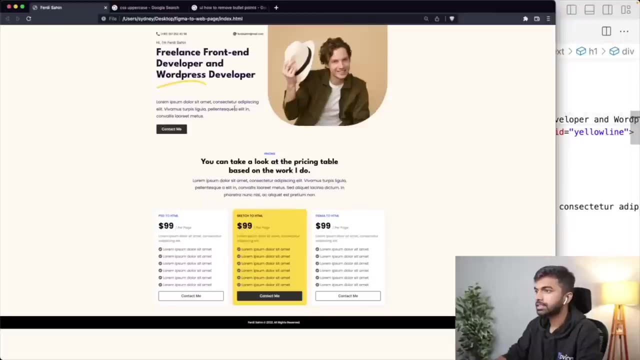 That's better. That is better, but it's still not doing it. I think maybe minus 80 PX still doesn't seem to be doing it. Well, what if we put this in a div? So this is where you'll have to experiment. This is where it becomes like a fairly tricky CSS. 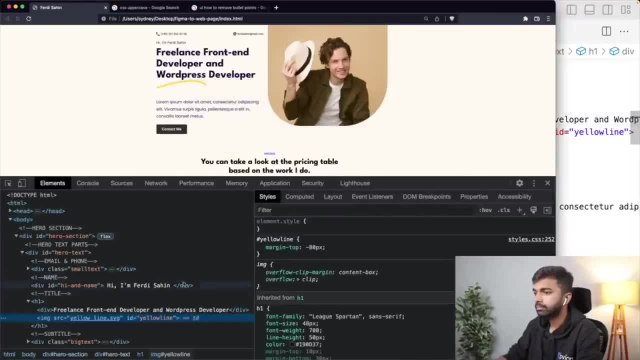 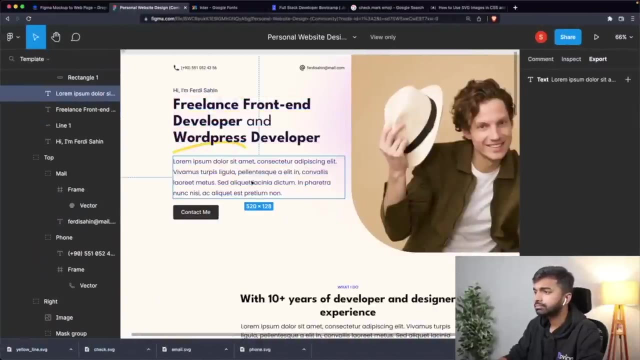 kind of thing to do And let's see if we can get IMG SRC ID yellow line. margin top is minus 80.. What if we said margin top to minus 200 pixels? still doesn't seem to be doing it, Okay. Well, I think I'll just give up at this point, But maybe what we 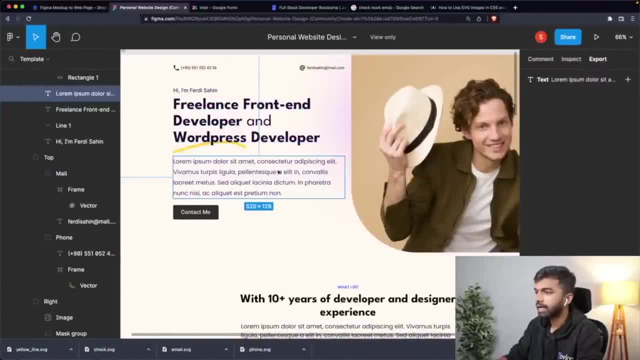 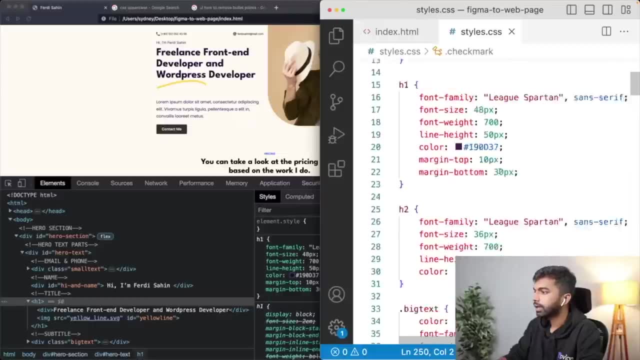 might need to do, then, is we might need to adjust some of these gaps, because now we no longer need this margin below the H1.. So I can go back into H1 and I am going to remove the bottom margin, which is 30 pixels. 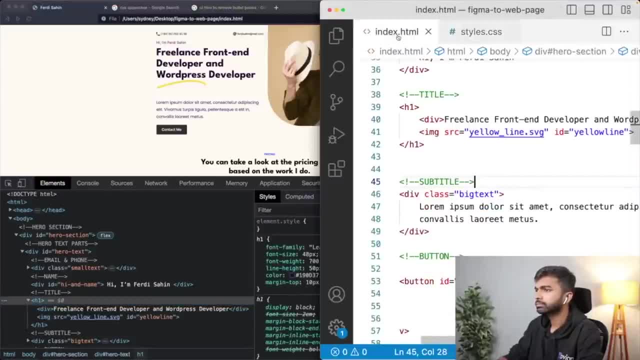 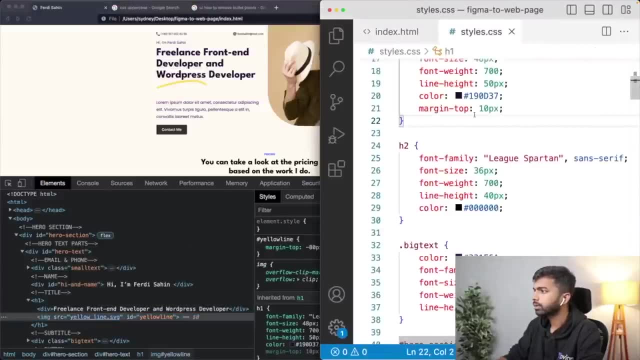 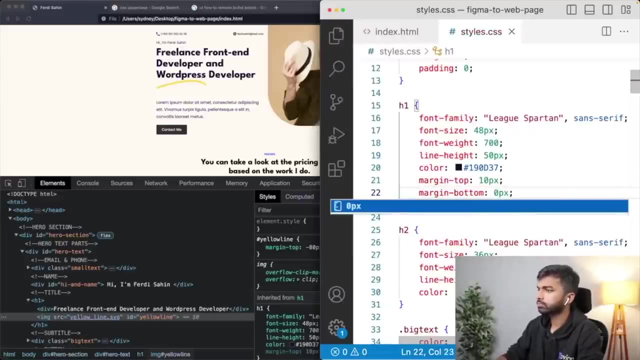 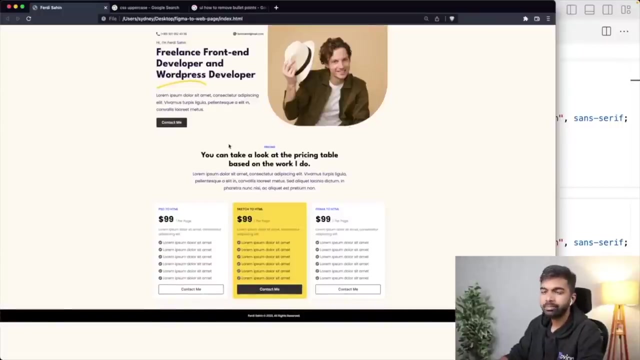 Yep, Let's see Now. do we still have a bottom margin here? No, Oh, we do, And I'm just going to set margin bottom to zero. Yeah, So that is close enough. There are other styling properties that can be used. 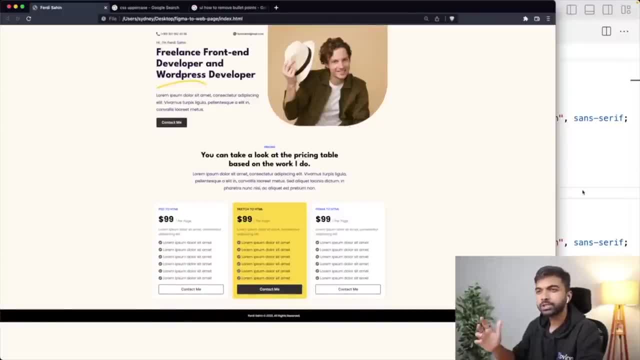 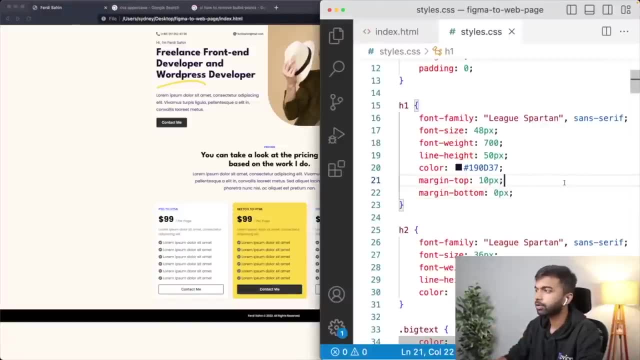 to achieve exactly what we are looking for. You can use something called position absolute. I'm going to use position absolute, I believe, position relative and absolute, and then you can set exactly where it is from the top. that might be able to do it. Let me give it a quick attempt. 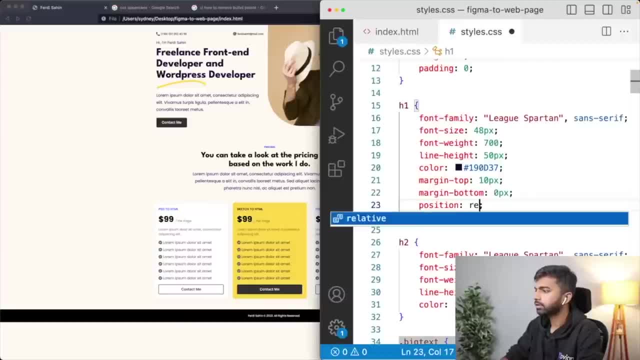 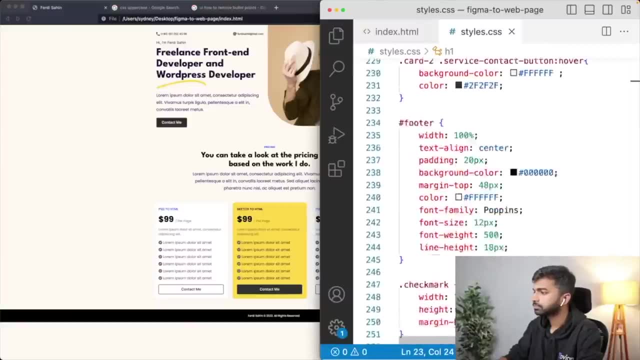 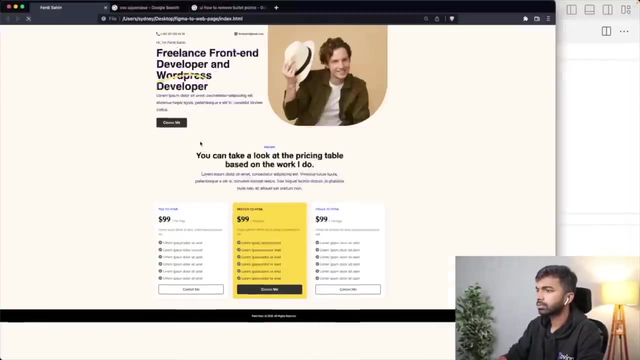 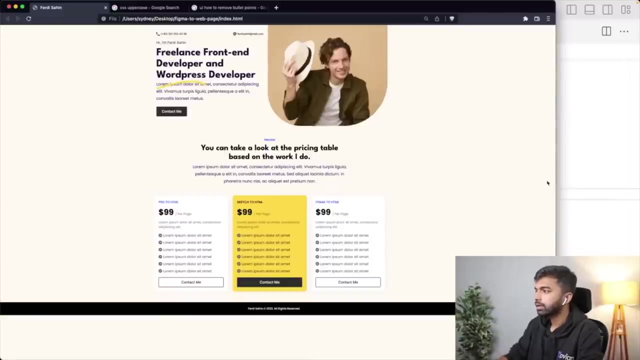 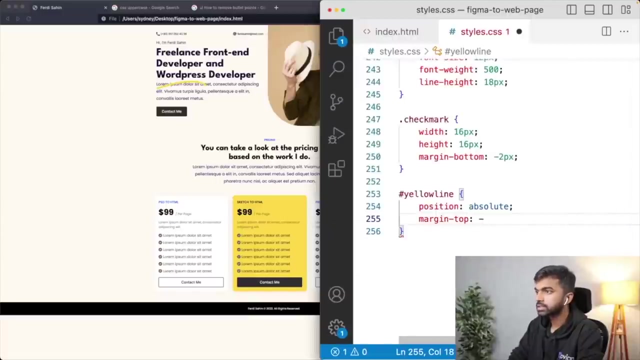 Position absolute or position relative. here And here I'm going to give it position absolute. Okay, That is doing it. Probably I probably don't need this And yeah, now I can say margin top minus 10px, probably like that. And if I want to, if I want it to appear behind the text, 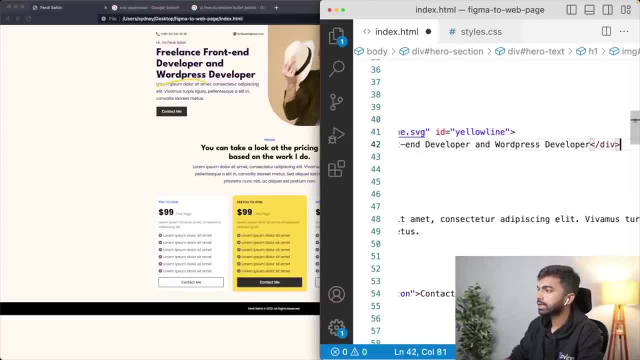 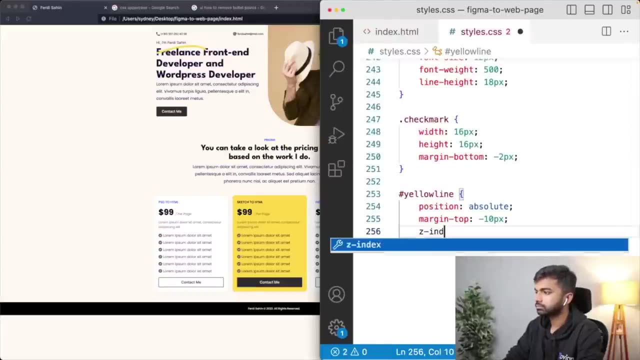 I need to put the text as the next thing here and not the first thing. Well, or we could use something called Z index. So, again, Z index is minus 10.. Let's say something like that, But it shows up behind the text. Okay, this is good. 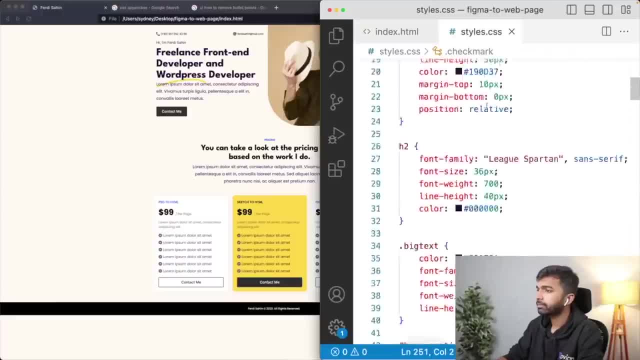 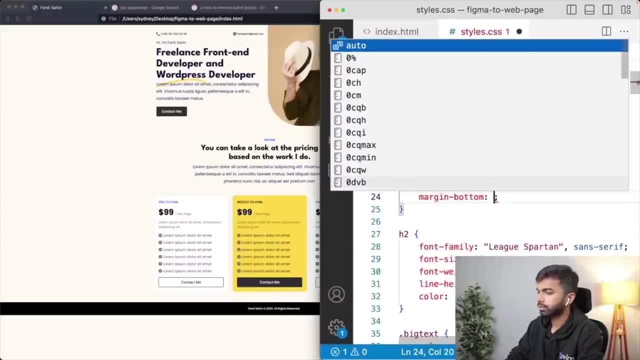 Now we can probably add back that H1 padding that we had. So let's see, we had a margin bottom: 30px- 30px- 30px- 30px- 30px- 30px- 30px. 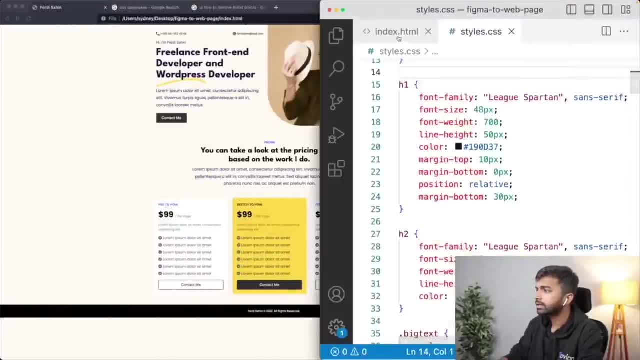 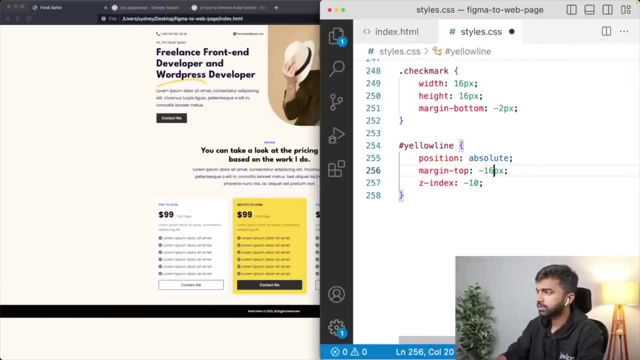 Yeah, so now this is almost exactly. okay. it's a little higher the yellow line. instead of it being minus 10px, maybe we can go minus 15 px. Yeah, and now it's almost exactly what we're looking for. 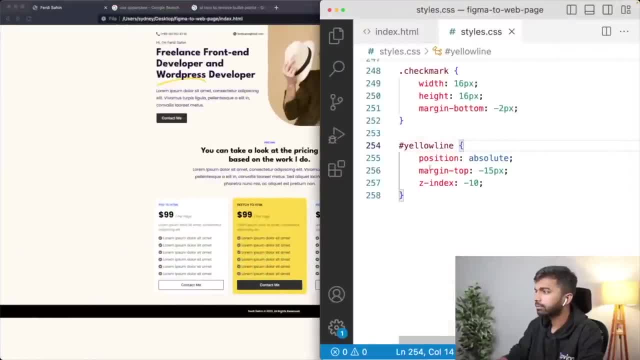 We have WordPress developer and we have WordPress developer. So what you can do is you can have a position relative on the parent, position absolute on the child, and then you can move it around anywhere within the parent. Okay, So what you can do is you can create a position relative on the parent, position absolute on the child, and then you can move it around anywhere within the parent. Okay, that's great. 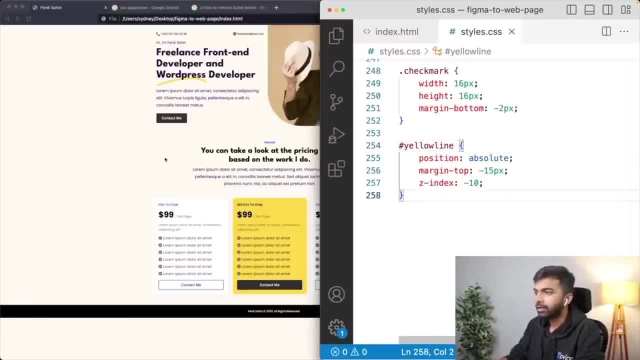 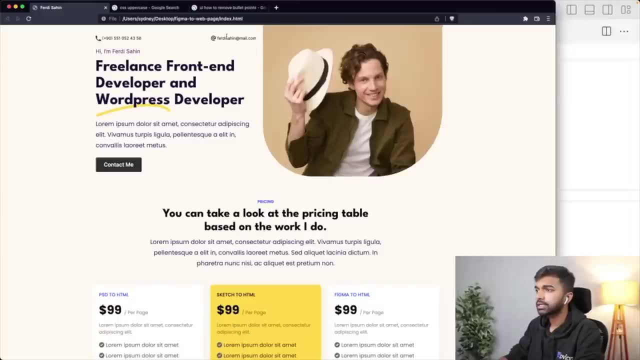 Okay, So that's just something that you can do in case you need to achieve layouts like these, but otherwise, this is looking good. I think I'm going to stop here. There is a title section, There is an email section and we can, of course, hyperlink this. 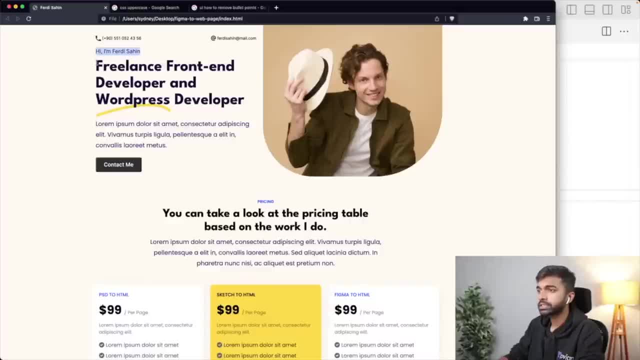 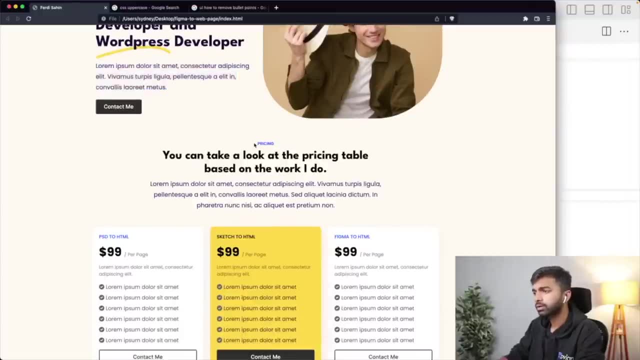 We can hyperlink this. All of those things are possible. Uh, this is looking good. Freelance runtime web developer and WordPress developer And this is looking fine. Contact me, It looks good. Uh, pricing- the boxes with pricing and then the layout. 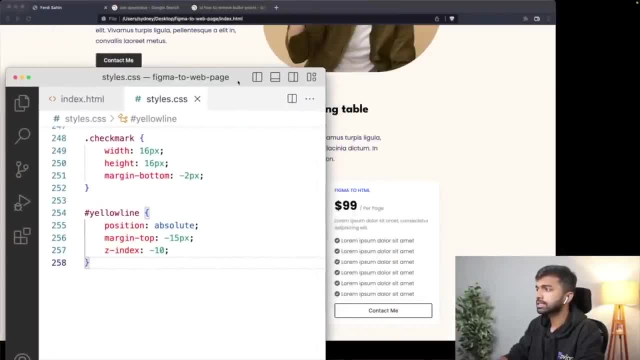 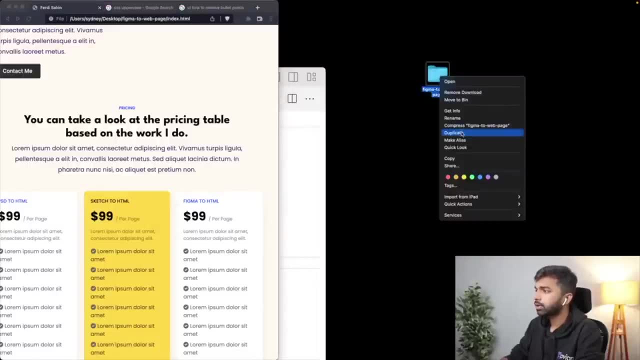 The last thing I'm going to do is I'm going to quickly show you how to deploy this, in case you are going to share this with somebody. So here's what you can do: Just zip it up. go to compress Figma to webpage. just zip that up. 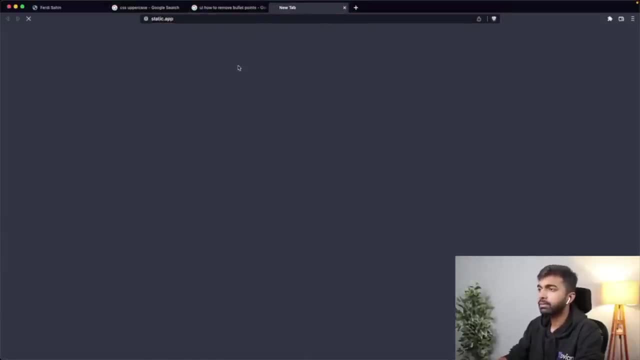 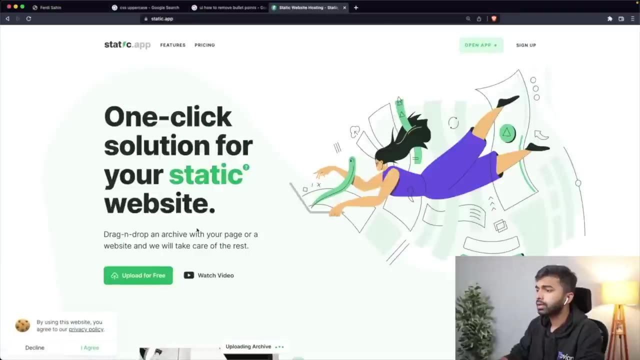 And we're not going to use gate or anything here. I'm just going to use this free platform called staticapp. Let me just sign out here so that I can show you: Yeah, And your staticapp allows you to just take a zip file and you can. 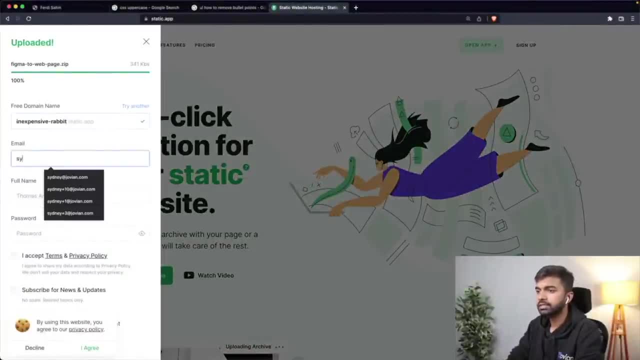 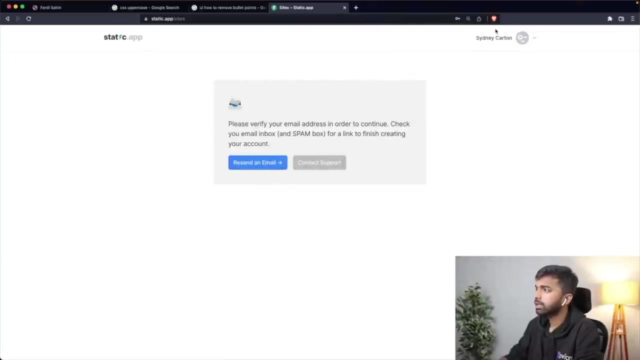 upload that and deploy it. inexpensive rabbit. Okay, Let me just add Sydney, plus 99 at joviancom. Okay, Okay And let's, yeah. so this is a site where you can upload a zip file and then you can just you'll. you'll have to verify your email. 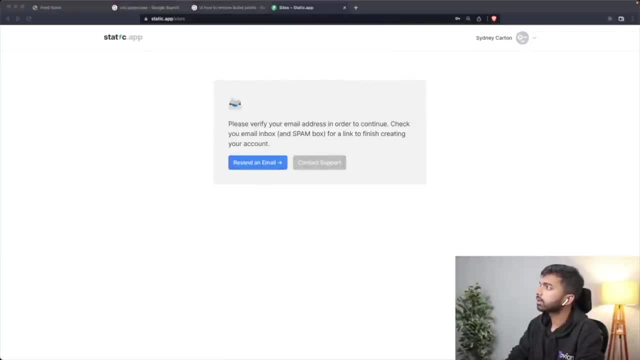 Let me go ahead and do that right here, doing it on another screen here. Okay, I'm going to activate my email done And once my email is activated, it has taken the zip file and it has simply uploaded it on the crowd cloud. 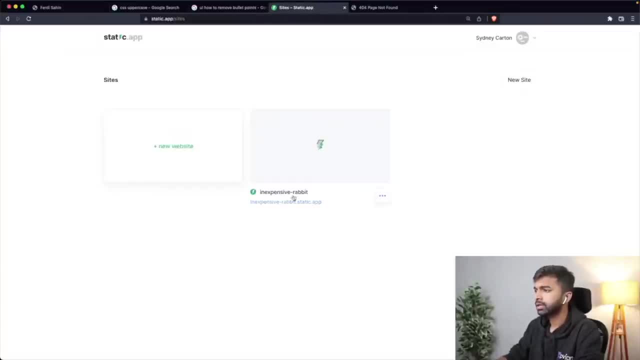 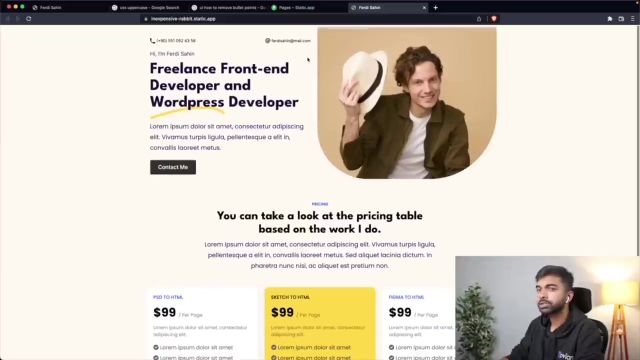 And it has given us this URL. It is. it takes a minute or two to set up, But at this point, yeah, it is still unpacking the archive looks like. Yeah, So this point, our website is deployed, and you can also then connect. 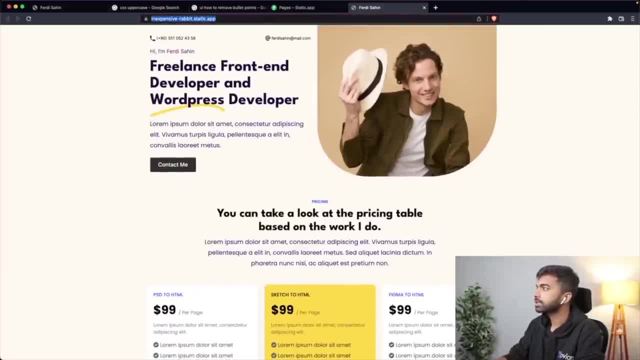 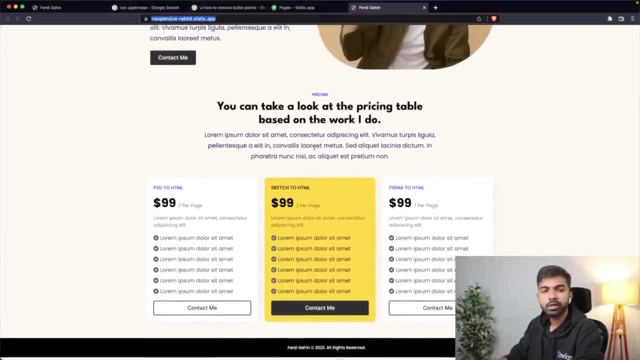 staticapp to your own personal domain. So I'm just going to share this link with you so that you can actually verify that this is. this website is actually deployed, but this is all that is. you have a layout like this, which is given to you in Figma. 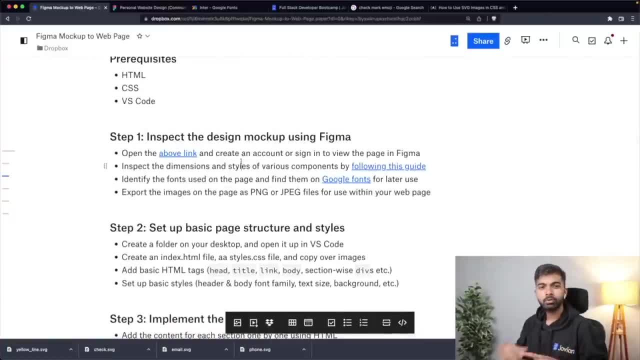 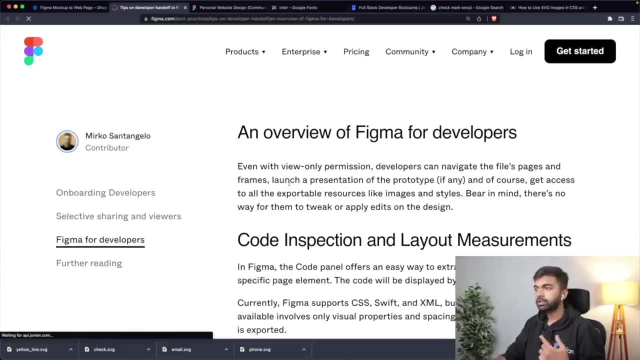 The first thing that you do is inspect the design mockup. You identify, okay, What are the different dimensions or different components- And there's a guide here that you can check out- which are an overview of Figma for developers and how developers can use Figma. 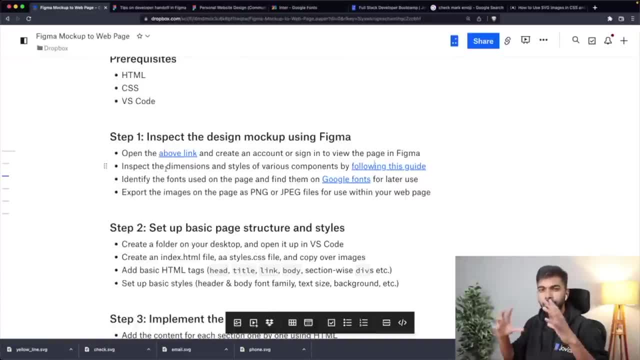 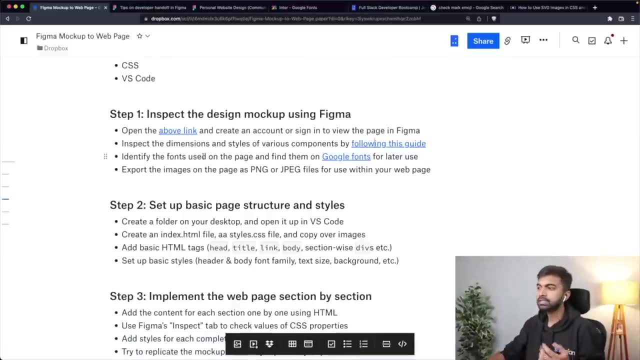 But the idea is you just inspect the design, You identify what are the various sections, You identify the fonts used on the page. You identify- you find them on Google fonts. You export any images or JPEG files that are being used within your web page. 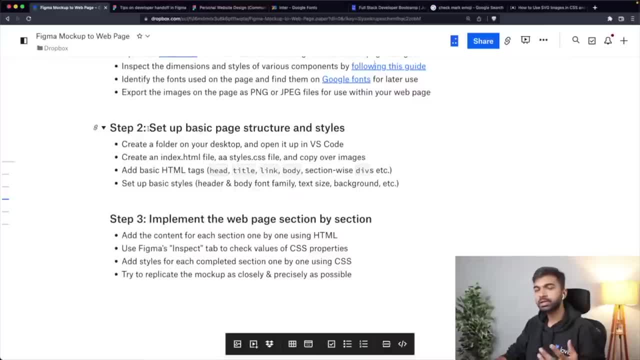 Then the next step, step two, is to To set up the basic page structure and styles. So you create a folder on your desktop and then you open it up in VS code, or if you're using Git or something fancy like that, then you can do that to create an. 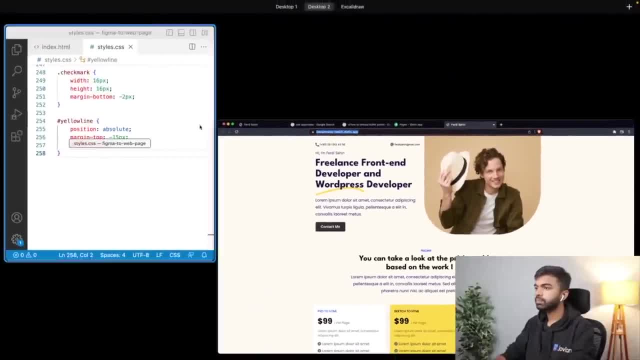 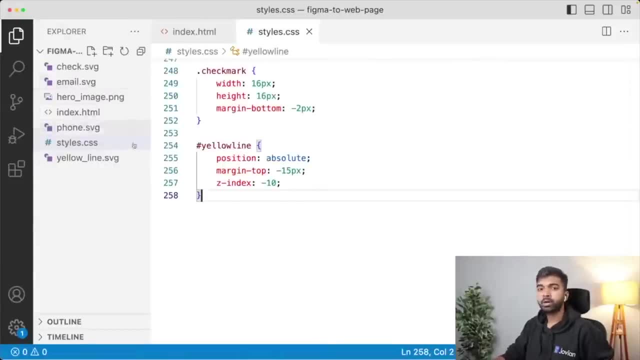 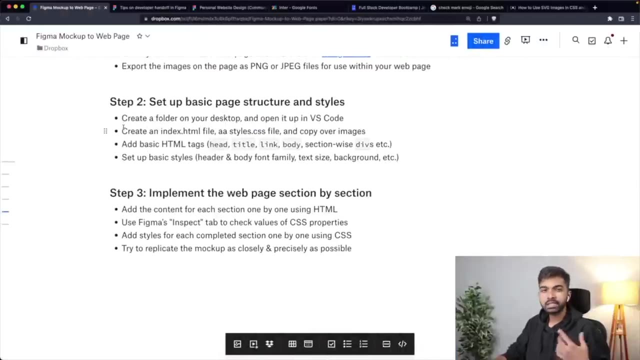 indexhtml file. create a stylescss file. That's what we have here. We have a indexhtml, We have a stylescss and copy over all the images that you need. So the hero image was the only image And then we had a bunch of these. then you add the basic styles. 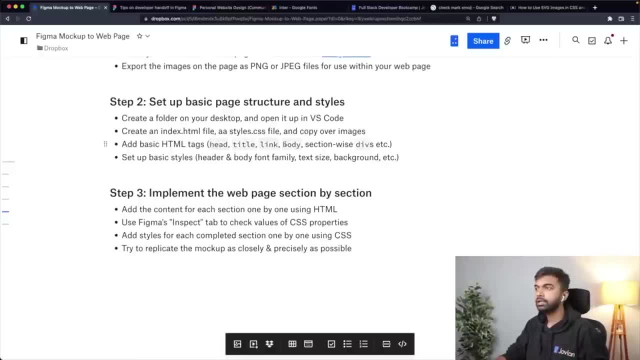 So you add basic HTML tags: head, Title, link, body- Uh, we added all of those first in our file. Then you add the various section wise div. So you create a div for each section, because each section, ultimately, is going to be a box on the page. 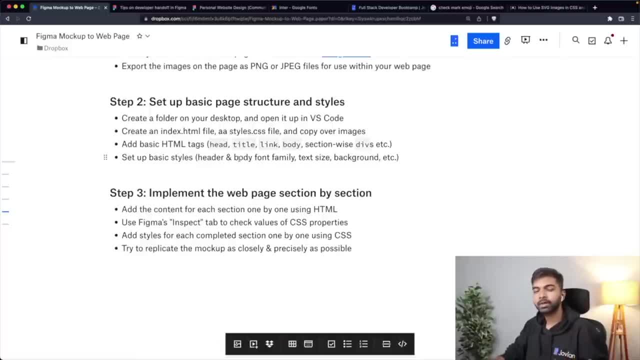 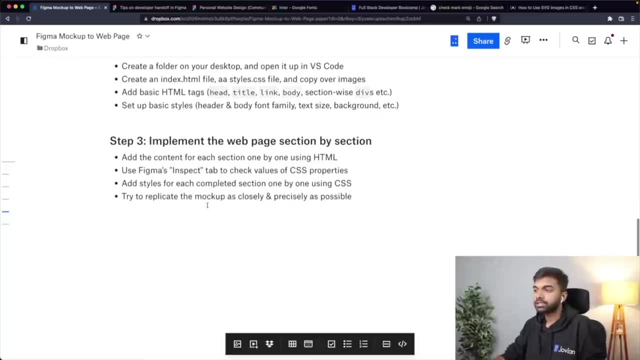 Then you set up some basic styles for the body, You set up basic styles for the header, You set up backgrounds, font families, text sizes, colors, et cetera. Then you go ahead and you implement the webpage section by section. 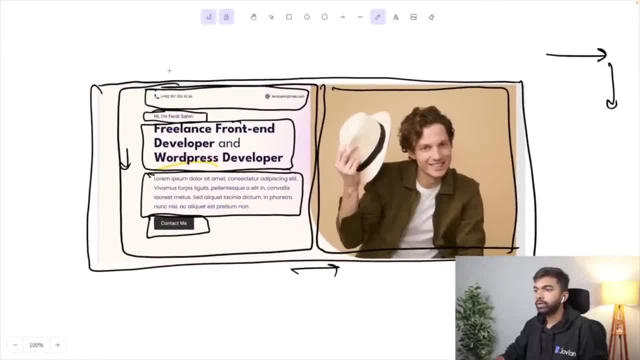 And the key there is to first identify in the box Whether the box is in a horror, whether things are arranged in a horizontal direction or a vertical direction. So you always want boxes and the box has to be, has to have something in a 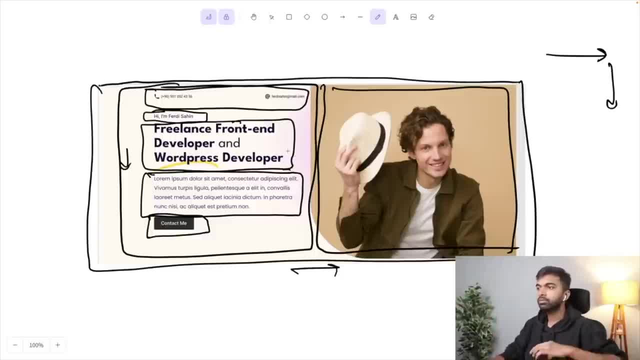 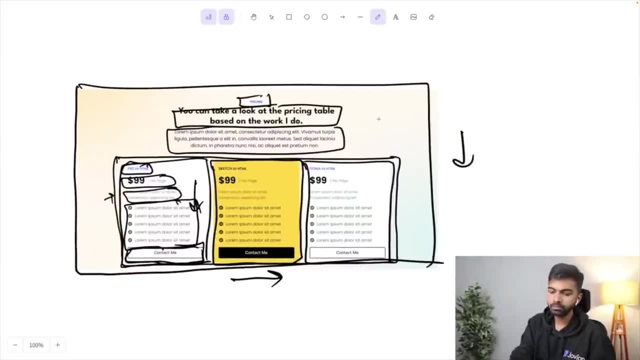 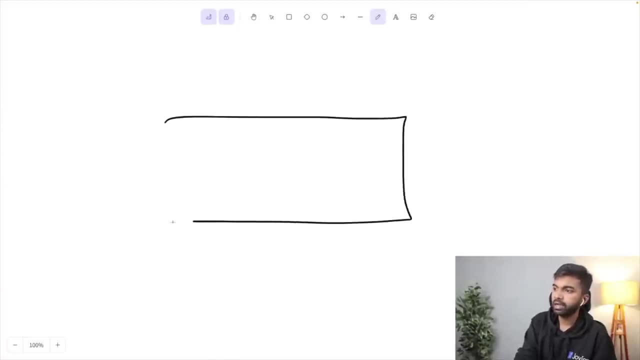 vertical direction or something in a horizontal direction, and then you then create boxes within boxes, right? So you're always looking to create a layout like this, where you have, Or a layout like this, where you have a box and then, within this box, one possibility. 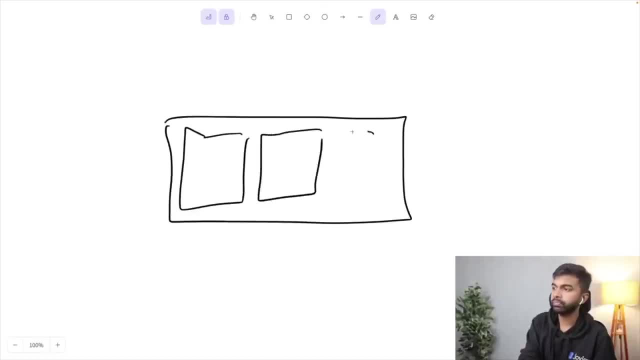 is that you have boxes that are laid out horizontally, like that. or the other possibility is that you have a box and within this box things are laid out vertically and so on. then, of course, again within that horizontal box, you can have like a bunch of vertical boxes like that, right? 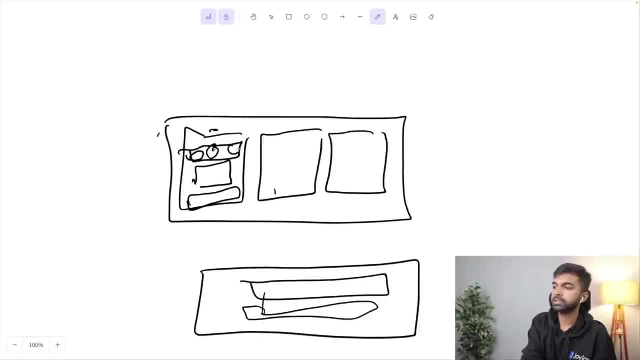 And then within each of those vertical boxes, you can again have a bunch of horizontal boxes. So if you start thinking of your web design as something like this, as a bunch of boxes inside boxes inside boxes, with each box having its children laid out in, 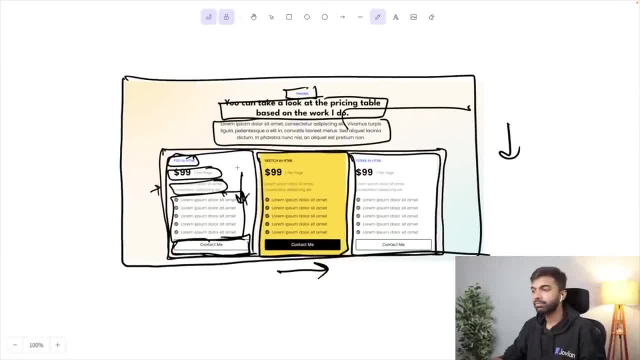 horizontal or vertical order. then your web design becomes really simple and you'll never run into a lot of the CSS issues that often plague web developers. So in this case, for the pricing table, we had a vertical layout first, So the box, box, box and then a big box. 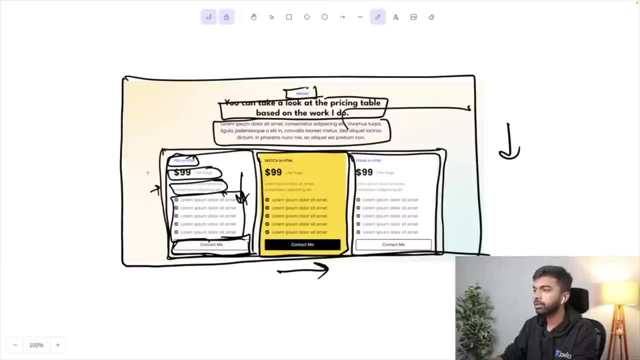 And then inside the big box at the bottom, we had a horizontal layout box one, box two, box three equal width. That's where for horizontal layouts you use display flex. And then for each of These inner pricing cards we also used a trick where we added another. 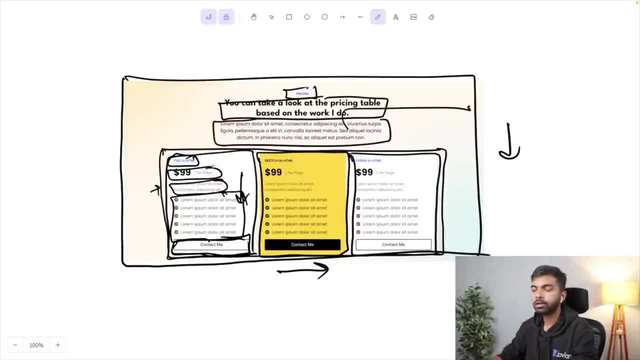 inner div, which will have its own radius and border, and all so that the outer divs were just for creating the bits and the inner divs were creating the cards, and then, in the pricing card, we have a horizontal vertical layout. Okay, So that's all you need to know. 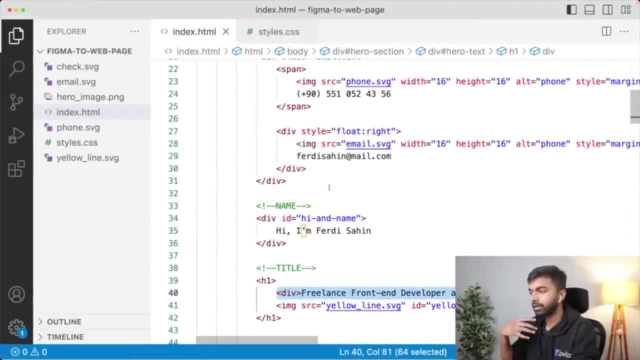 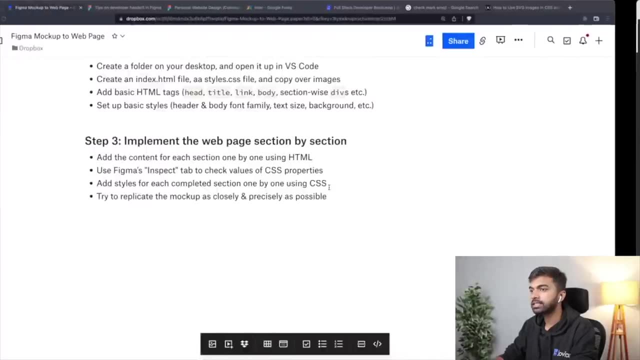 That's all you really need to know in terms of taking a web design and then converting it, or taking a web design mock-up and converting it into a webpage. Of course, there are these special cases Like this, where you have to figure out how you're going to add that. 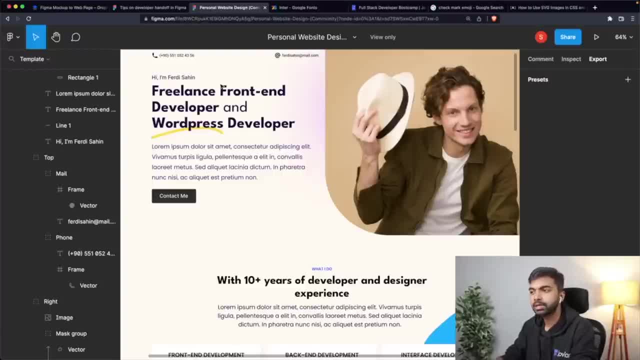 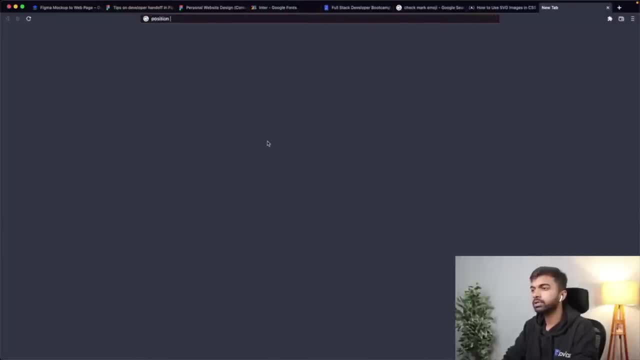 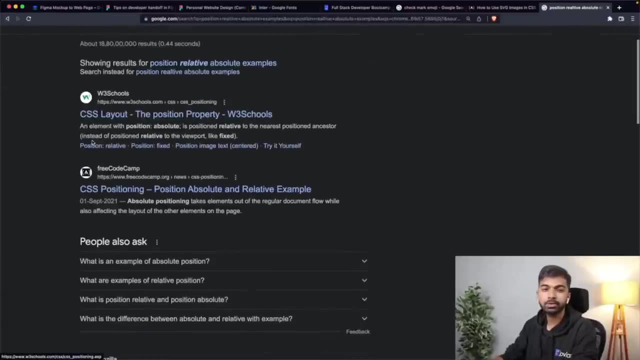 But the way you do it is by using some negative margins here and there, maybe using a position relative for the parent, absolute for the child. You can always just search position relative, absolute examples And there are a bunch of tutorials on this. Like nobody knows exactly how to do these things. 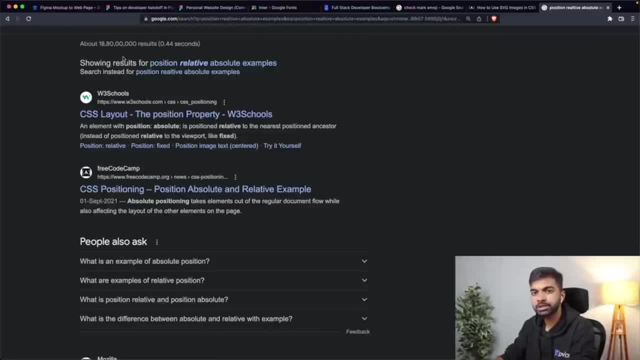 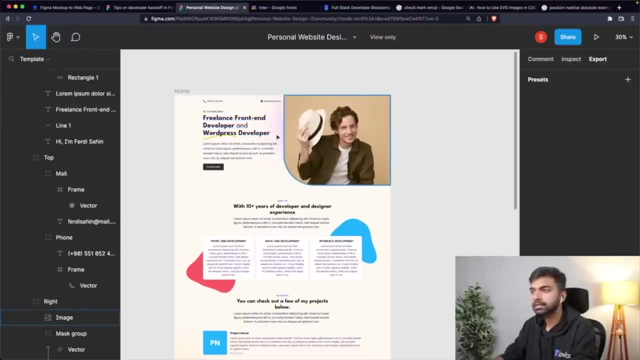 You have to learn, you have to search for them, and position is generally one Thing when you have, like, one thing behind another that you can deal with. So similarly, you can maybe get this one element, this this nice glow that you have. 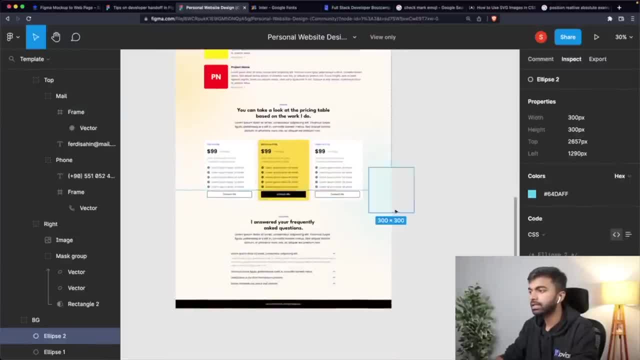 here. you can get this element somehow. you can try to get this element, this glowing thing, and you can export that ellipse as a PNG file or an SVG file, and let's see, Yeah, And then you can just incorporate that within your code as well. 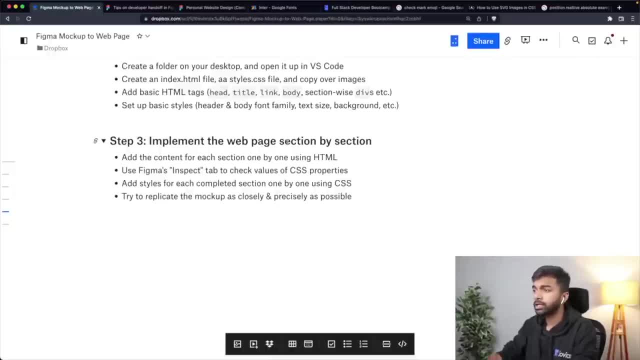 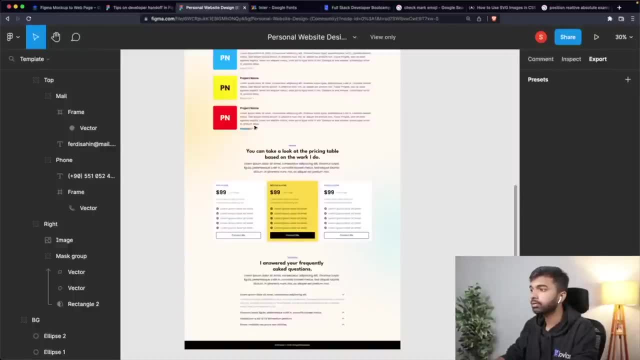 Okay, All of that is doable, So, yeah, So you add content for each section one by one, using HTML, by using that box structure. Then you use Figma's inspect tab. So remember, here you select anything and you can see exactly what properties it is using. 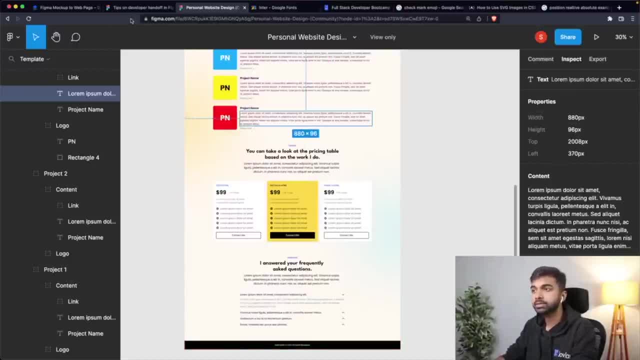 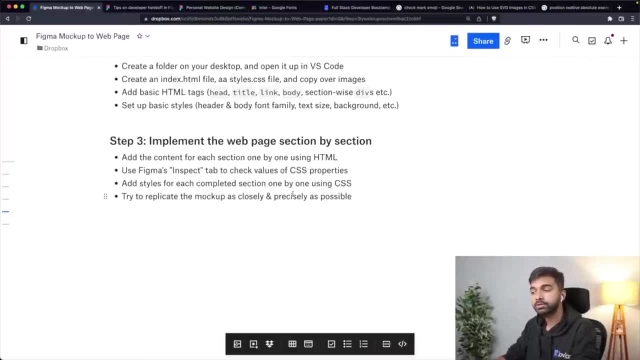 It's not that you will be able to copy these over directly. You may have to make some changes to it, but you use Figma's inspect tab to check values of CSS properties, add styles for each completed section one by one using CSS, and then try to replicate. 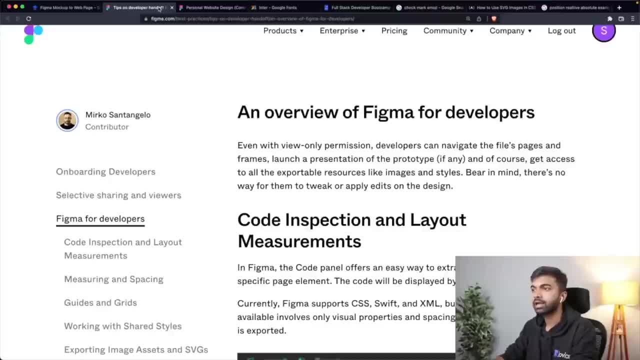 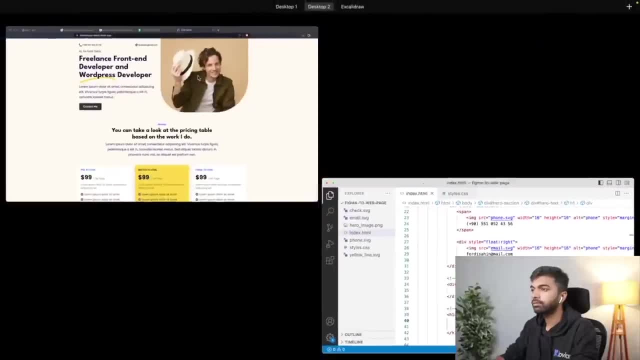 the mock-up as closely and as precisely as possible, And that's where we get into these minor details. Like over here. we have this ad character which is vertically centered, So maybe We can achieve the same thing over here like that. 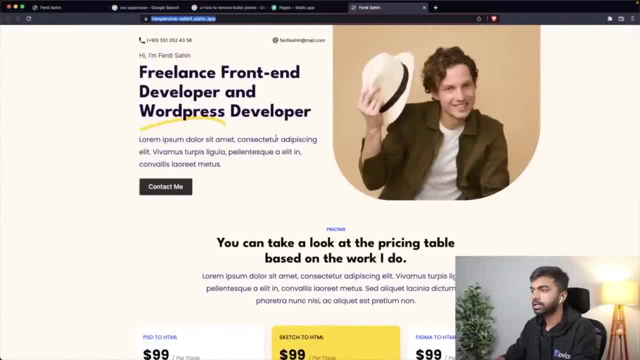 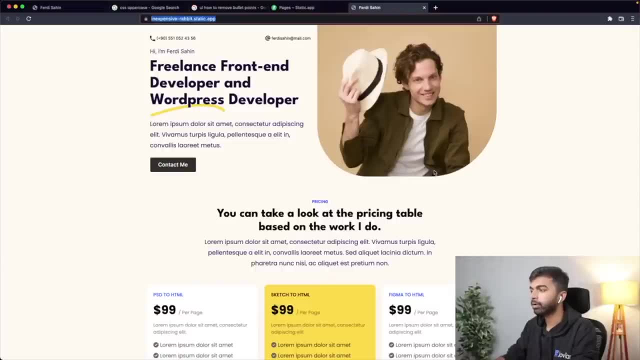 And often there may be some trade-offs we will have to make when you actually go ahead and implement the design. For example, we reduce some spacing here. We decided that we are going to center the image on the page and add a border to it, because otherwise it just looks a. 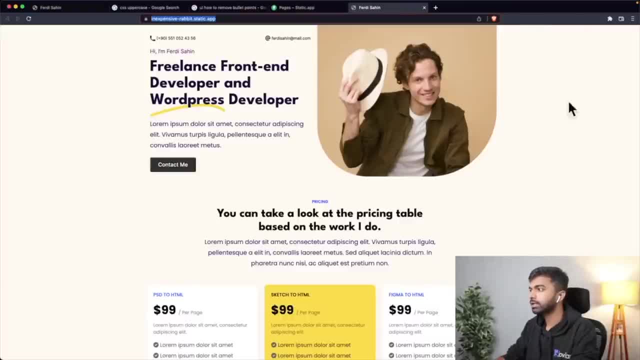 little odd that the image is not only sticking out, but it's also. then there is some space on the right which is empty. Okay, So that is everything that we're going to cover today. So thank you for joining, And there are a bunch of. first of all, I would love to know how did you find the session? 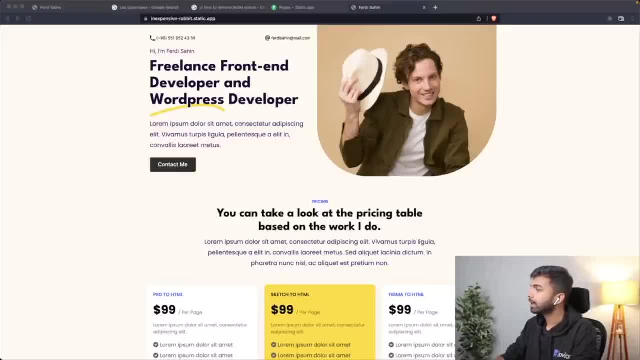 You can drop a line in the chat and we'll see. but there are a bunch of comments or questions as well. Let's see How do we get the Figma file? We will share. we will add a link in the description, but let me also share that link with you right now. 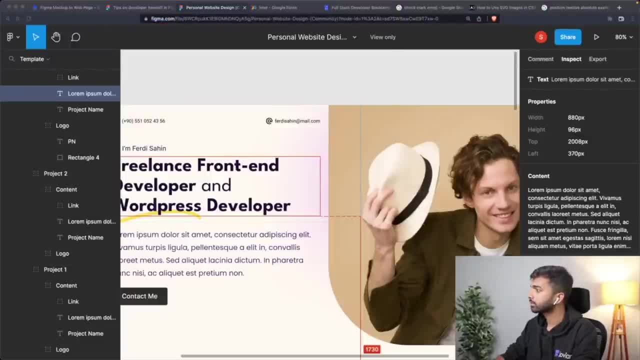 So this is the Figma file that you can use. Then you should use the button Tag inside an a tag for Amelia. Okay, So that was a nice tip that I can actually put the button tag inside an a tag. So that's great. 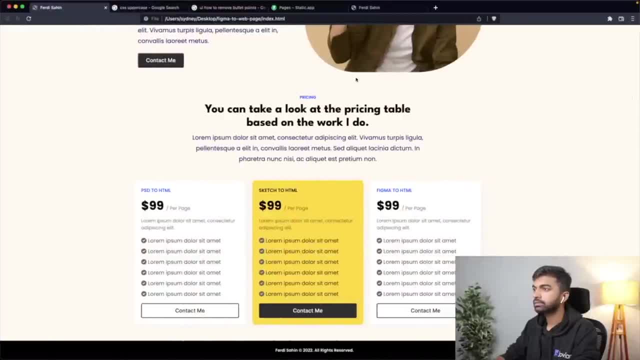 I will definitely do that, Or we can actually just fix that right now. I believe that's okay. It's okay, We are out of time. How was? state is not added? Yeah, So we've added the hover state, not for this button. 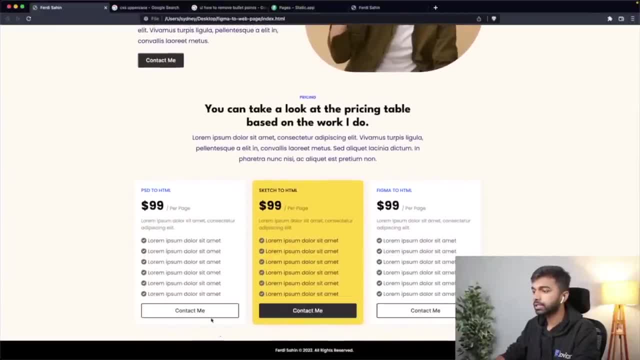 Yes, we should add it for this button also, but do you added the hover state for these buttons? Would you recommend to use live server so that you don't have to reload the website? Yeah, So you can use VS code extension like live server. 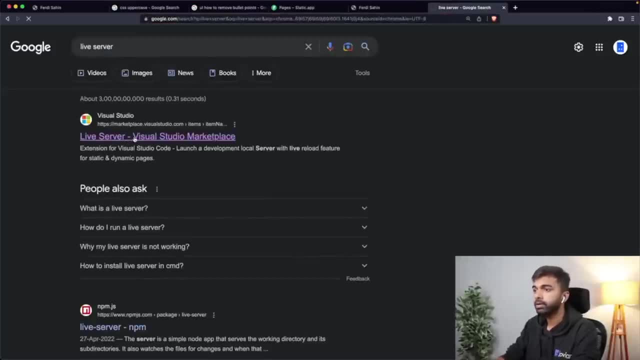 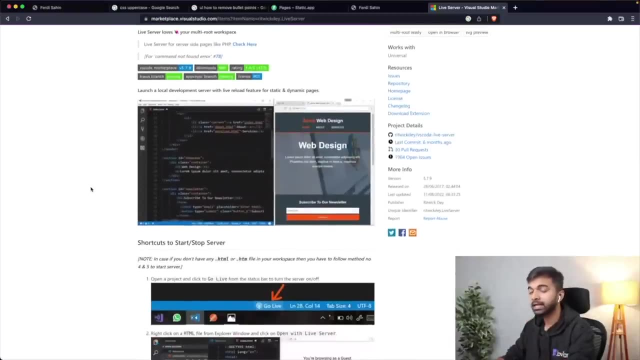 So there is this VS code extension called live server. You can use it If you're using VS code on the cloud, like GitHub code spaces, or you can also use it locally, And the benefit is that anytime you make a change to the file, it automatically reloads the page. 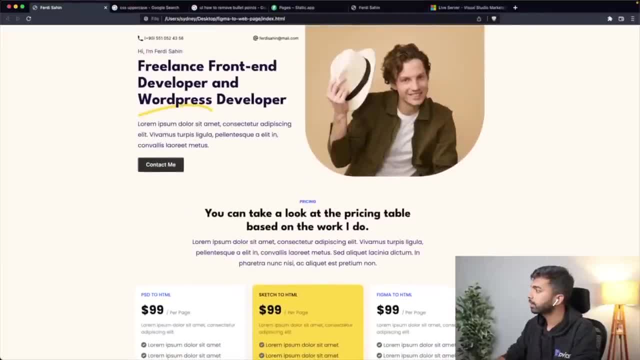 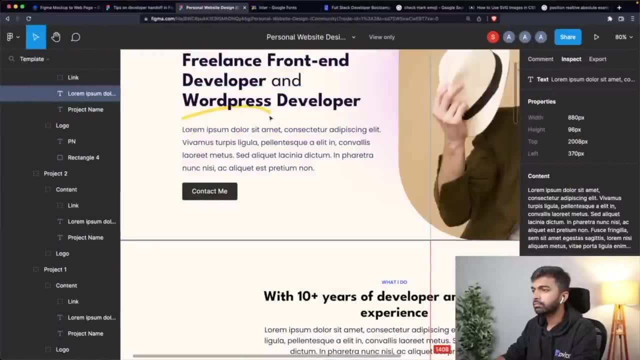 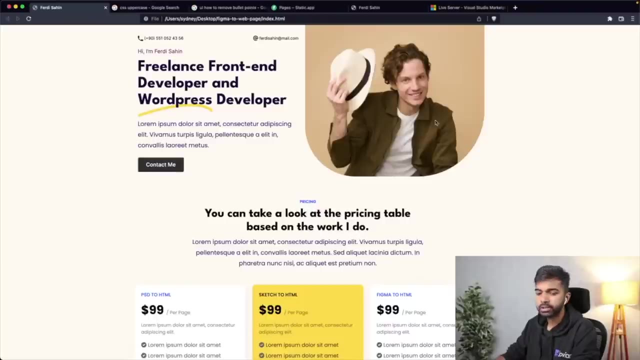 So you can use that too. I just wanted to keep things simple for today. and yellow line rotated 45 degrees. Well, it's not rotated here, but yeah, Okay, Okay, Okay, Okay, Perfect. Well, I think we will close at this point. 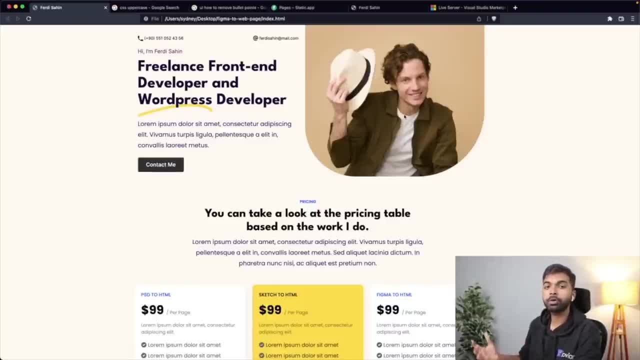 So thanks a lot for joining. I hope you enjoyed this tutorial And if you want more tutorials like this, come join our WhatsApp community. We'll drop a link in the chat. It's just joviancom slash WhatsApp So you can join our WhatsApp community and you'll get to know about more future events. 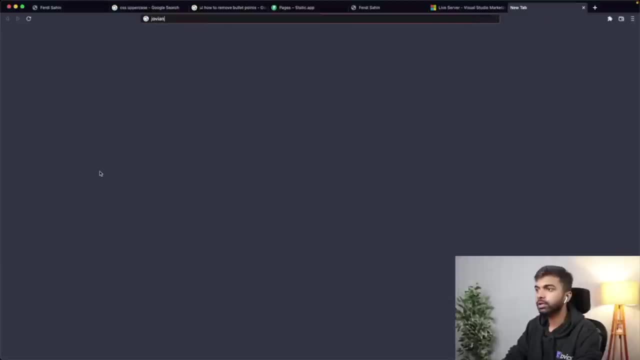 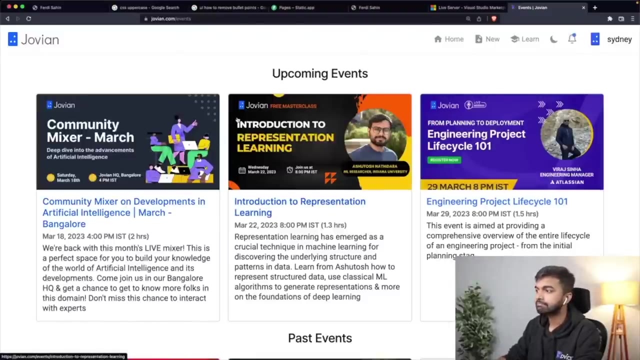 We have events happening every week, more or less. We can also just go on joviancom slash events and learn more. We can also just go on to our website and learn more about these events. So, yup, I hope that is helpful now and I'll see you next time. 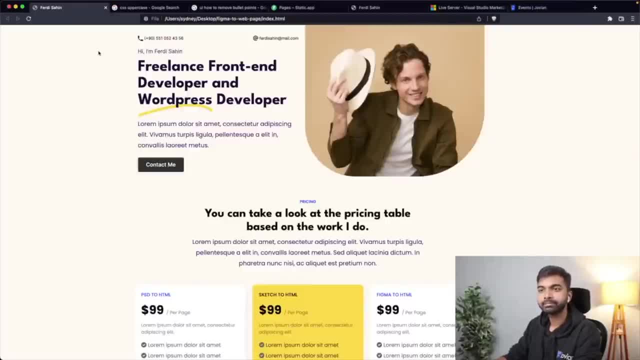 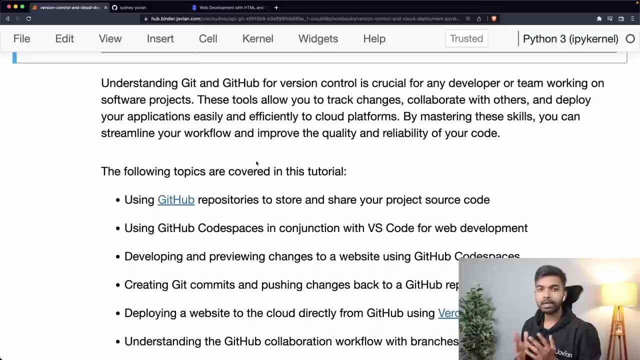 Thank you and have a good day or good night, Bye-bye. So let's get started. Understanding version control, Git and GitHub is crucial for any developer or any team working on a software project. So far, we have been building our websites just by setting up folders on our computer. 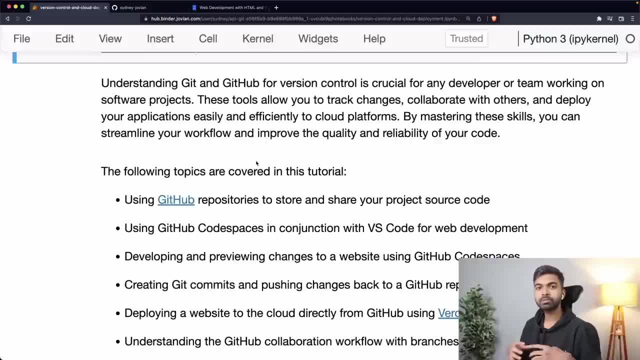 opening them up in VS code. But to professionally build websites you will need to track the code in a version control system. So these tools allow you to track changes. They allow you to collaborate with others, because you're typically not going to be the only one working on a web application or website. 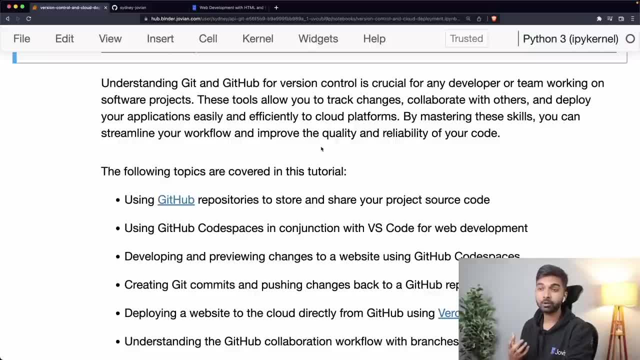 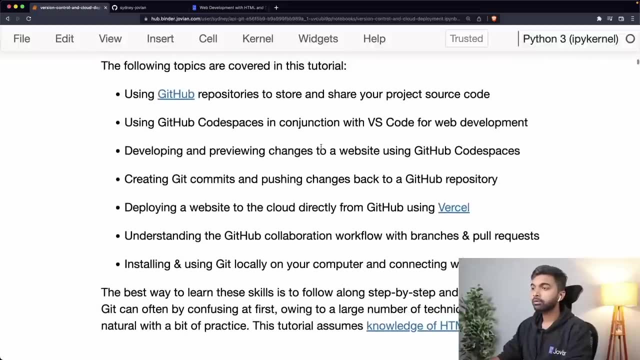 And they also allow you to deploy your applications easily and efficiently to the cloud, And by mastering these skills, you can streamline your development workflow. So today we are going to learn what professional web developers use when they're working on these projects. So, in particular, we are looking at these topics. 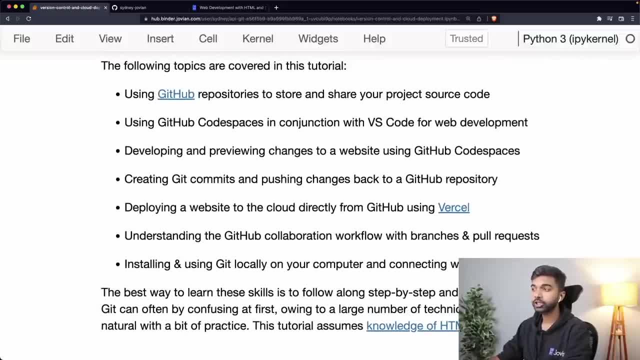 We will talk about using GitHub repositories to store and share your project source code. We will talk about using GitHub code spaces, which is an online code execution and online development platform in conjunction with a browser-based VS code or web development. We will talk about developing and previewing changes to our website using GitHub code spaces. 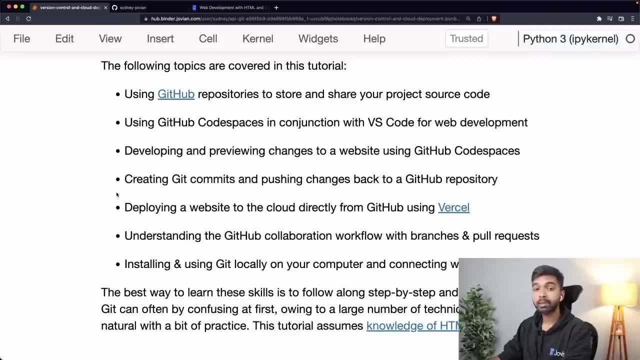 We will talk about creating Git commits- Okay- and pushing changes back to a GitHub repository. Then we talk about deploying a website to the cloud directly from GitHub using the Vercel cloud platform, And we'll try to understand the GitHub collaboration workflow, which. 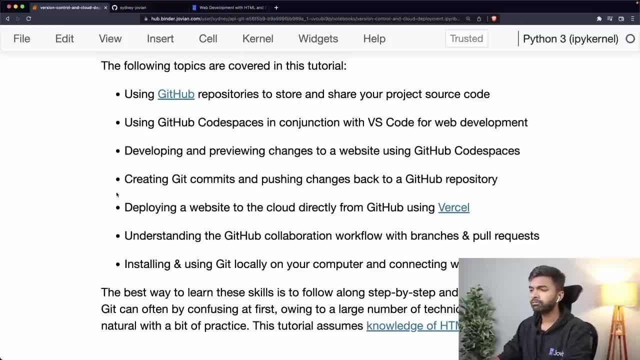 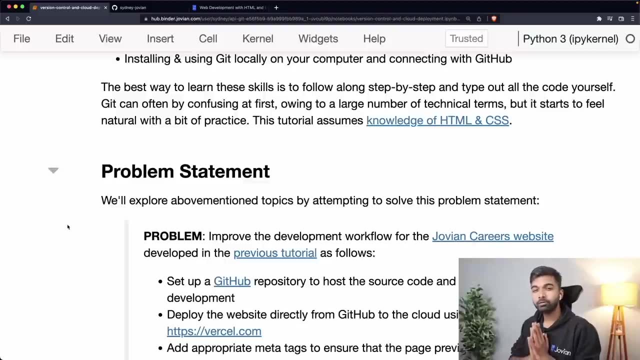 involves branches and pull requests. And finally, if we have the time, we will also touch on installing and using Git locally on your computer and connecting it with GitHub. Now, the best way to learn these skills is to follow along step by step and type out all the code yourself. Git can often be confusing at first. 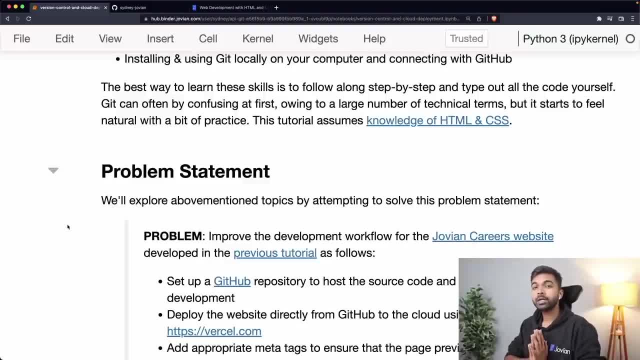 So I want to start with that disclaimer, because there are so many different terms that you will hear Git, pull, merge, commit, et cetera. but it starts to feel natural with a lot of practice And you will see us repeating the same flows over and over for the rest of this. 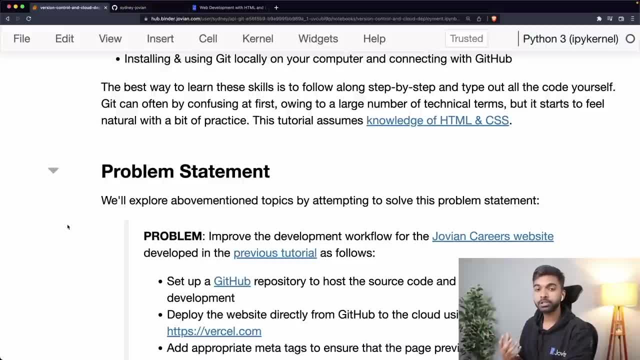 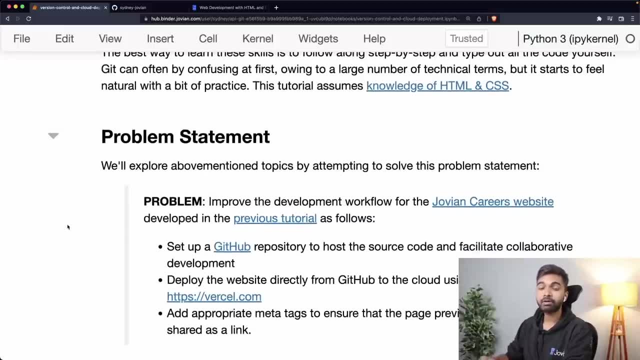 course and the rest of the program, But by the end you will become proficient in Git, whether you like it or not. Now, of course, this tutorial assumes some prior knowledge of HTML and CSS. So if you haven't completed the previous lessons, so if you haven't 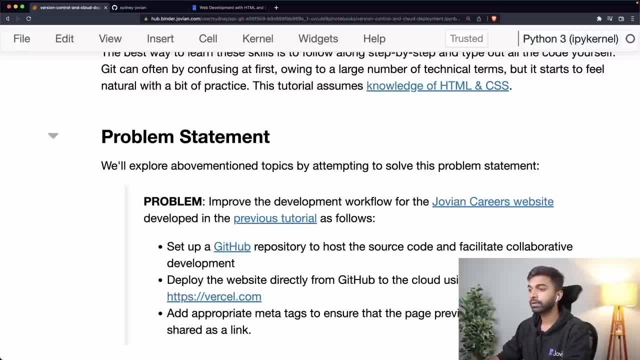 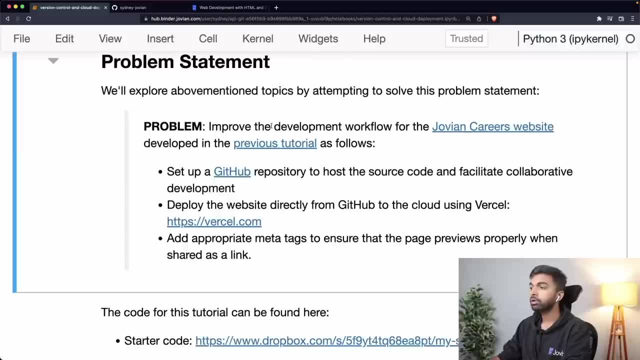 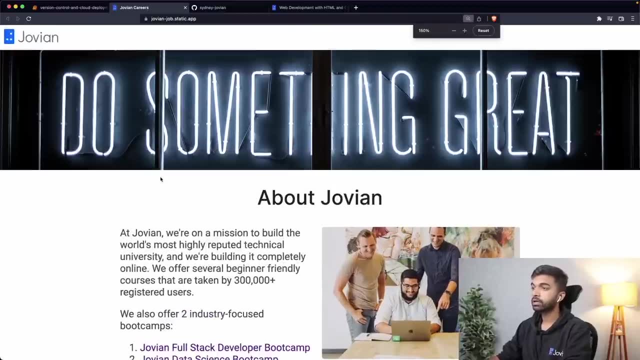 completed the previous lessons. please go ahead and complete them first, So we will explore these topics by attempting to work on a specific problem statement. We want to improve the development workflow for the Jovian careers website, So in our previous tutorials we've built this careers website, which 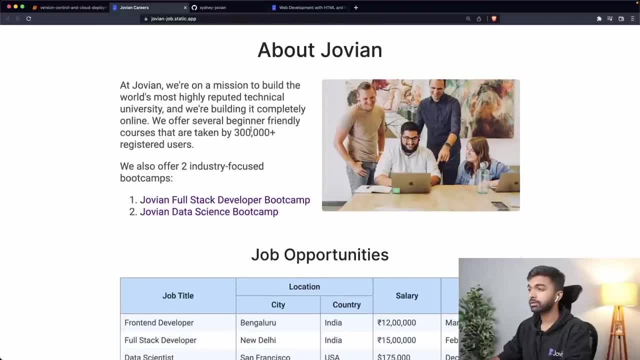 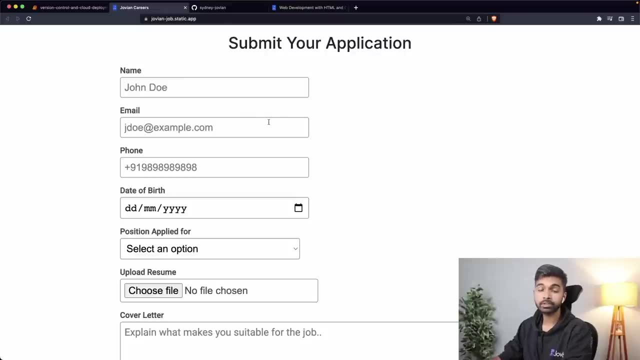 has a navigation bar which has this banner which has some information about Jovian, and image, which has a table showing the job opportunities. These are Jovian and it has a form where anybody who's interested in applying for a job at Jovian can submit their application. 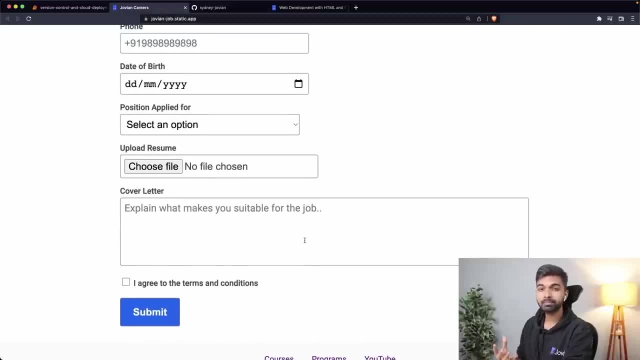 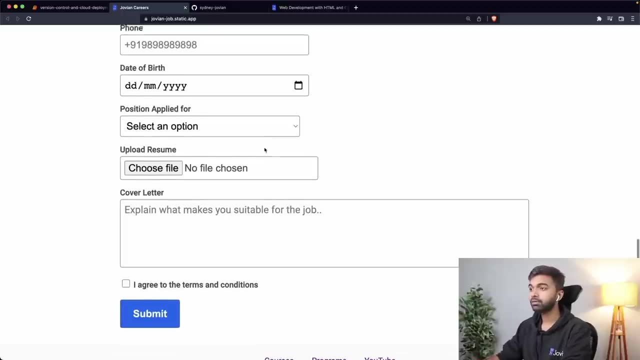 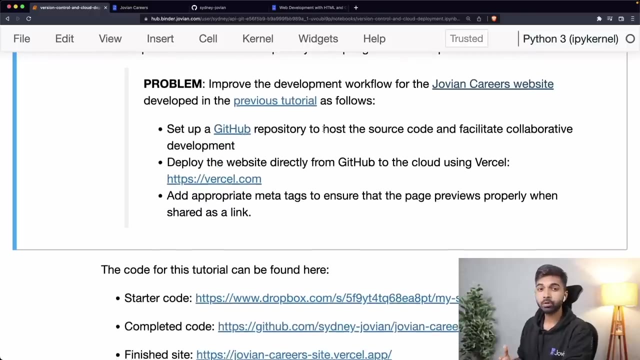 And finally, it has a footer at the bottom as well, And we built this by setting up a folder on our computer locally and then uploading a zip file to staticapp, And that is how we have this deployed version. So what we want to do is set up a GitHub repository to host the source. 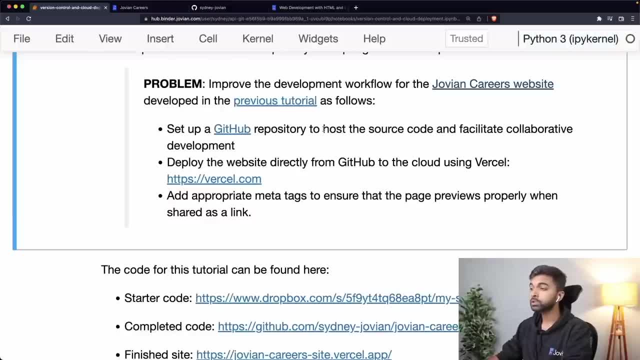 code and facilitate collaborative development. We also want to deploy the website Directly from GitHub to the cloud using the Vercel cloud platform, And we also want to add some appropriate meta tags, which we'll talk about today, to ensure that when you share this website with somebody, let's say on. 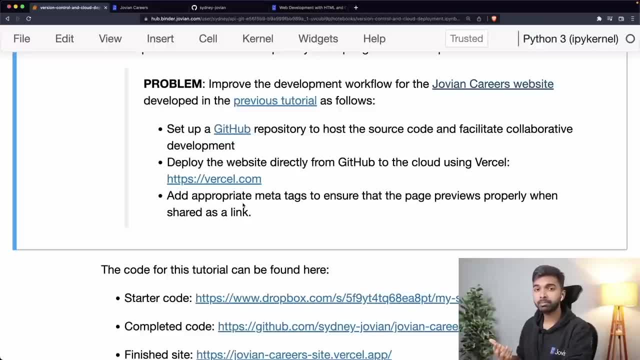 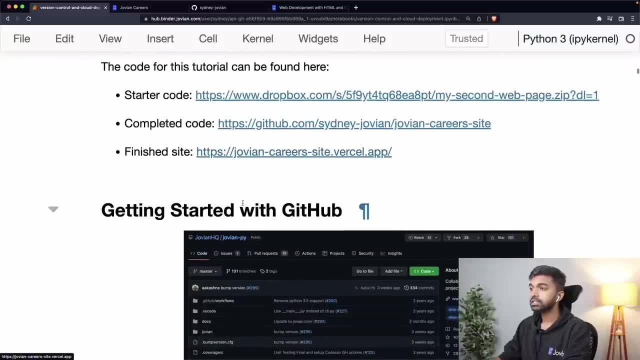 a social platform or as a link on a messaging platform, then the page previews properly. all of that is something that we'll try and cover today, So here is where you can find the code for this tutorial. We are going to start with the starter code, which contains all the code. 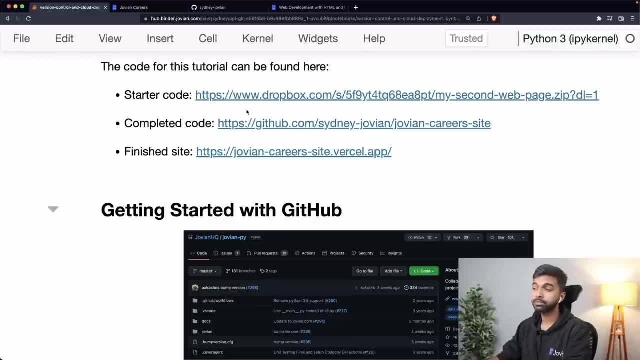 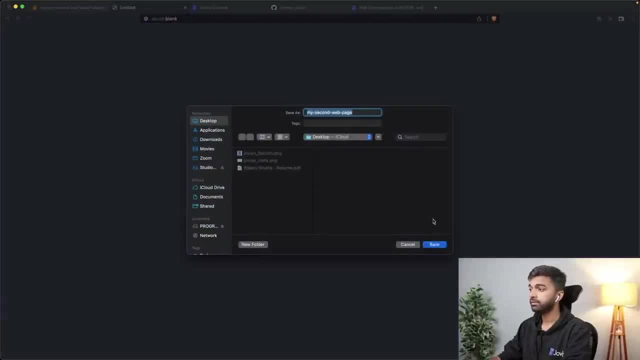 for this website that you're already looking at, which we have developed so far, until in the previous tutorials. Let me open up the starter code. This is going to be a zip file. I'm just going to save it here on my desktop. 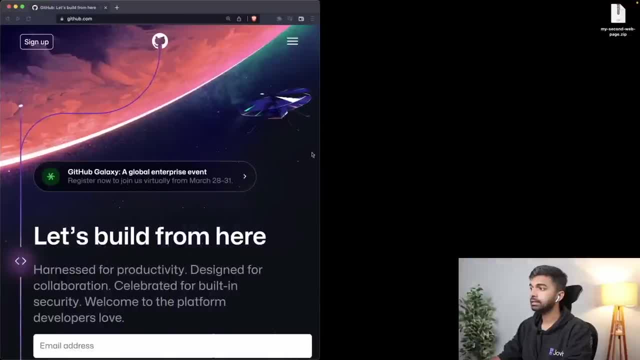 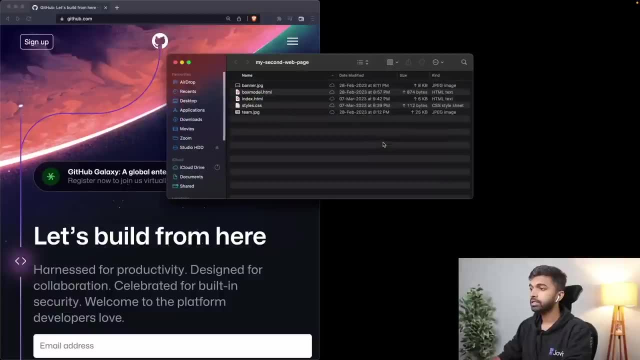 And once it's downloaded I can. then you can see here it's downloaded on my computer. I can then just decompress it. So now I have this folder. So in this folder I have the index or HTML file. I have a couple of other styles file. 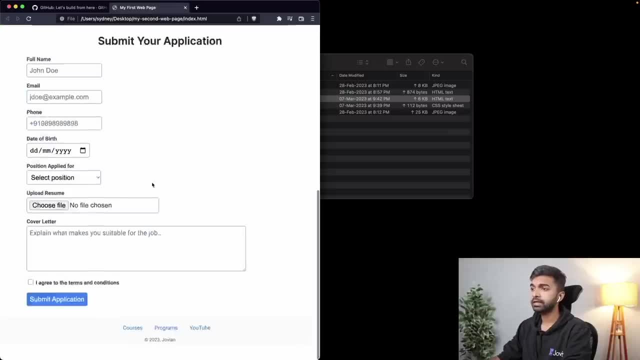 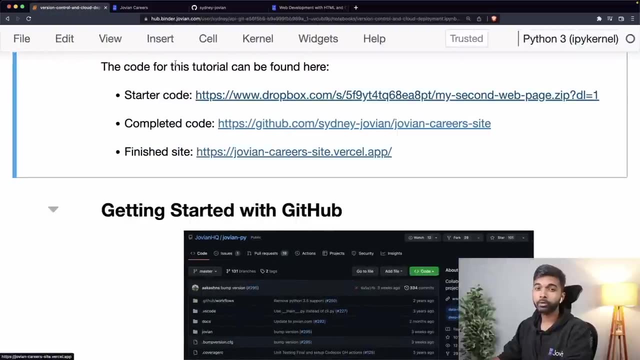 I have a couple, I have a couple of images, and this index or HTML file contains the actual application page, the Jovian careers page. Okay, But of course we are not going to do this development locally. We are going to do this development now using GitHub. 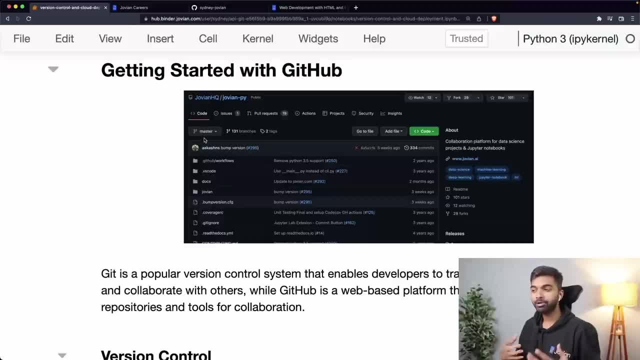 Now I'm sure, if you have, if you are pursuing web development, if you've done any programming, you must have heard about GitHub and you must have also heard the terms Git and version control. So first I just want to demystify these terms before we start using them. 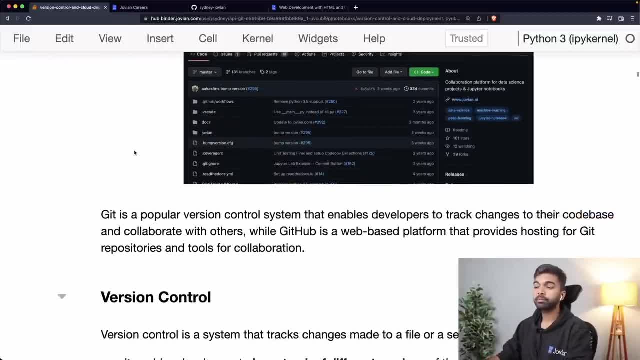 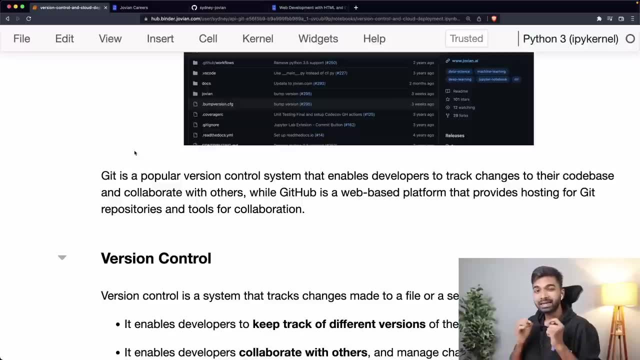 Now, Git is a popular version control system which enables developers to track changes to their code base and collaborate with others, and GitHub is a web-based platform that provides hosting for Git repositories and tools for collaboration. Okay, So let's break down each of these terms one by one. 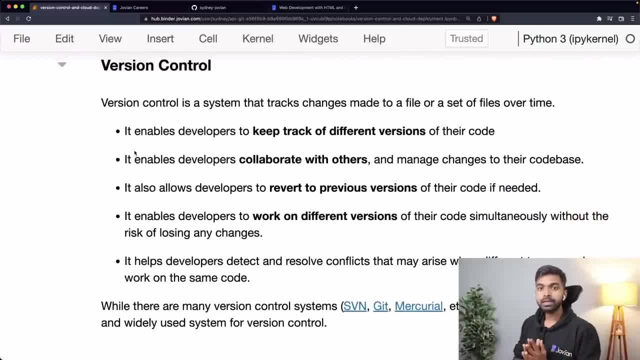 What do we mean by version control? Version control is any system that tracks changes made to a file or a set of files or a project, So it enables developers to keep track of different versions Instead of you having to create multiple copies saying V1,, V2,, et cetera. you can. 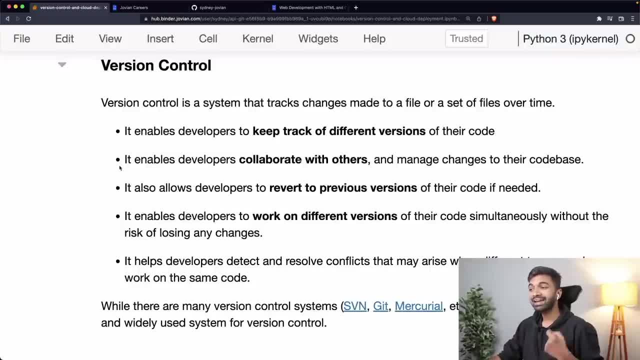 just put everything into a version control system systematically. It also enables developers to collaborate with others, so that you can have one common version and two people can build off it. Then you can bring those changes back And sometimes, when required, it also allows developers to revert to previous. 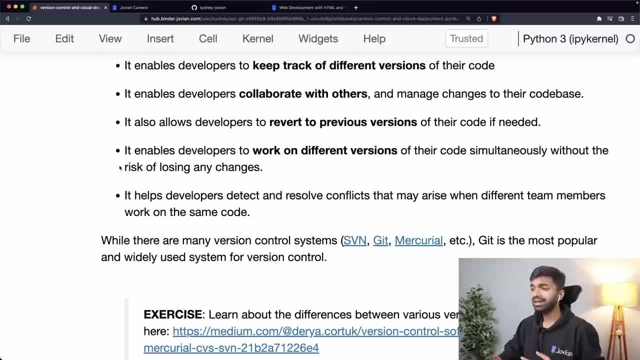 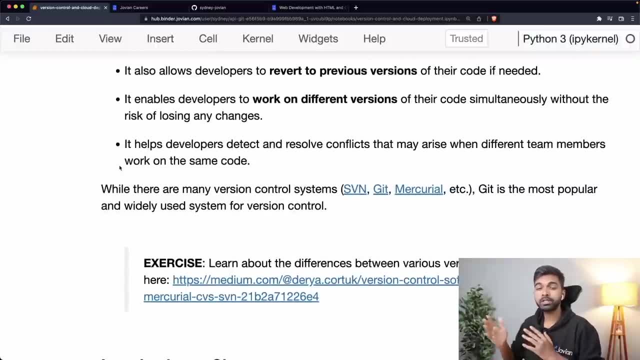 versions of their code if needed, And it'll enable developers- Developers- to work on different versions of their code simultaneously. So, as a developer, sometimes you work on multiple features at a time, And again you need a version control system for doing that. 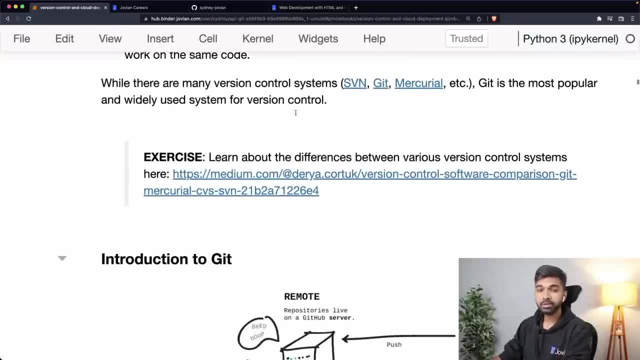 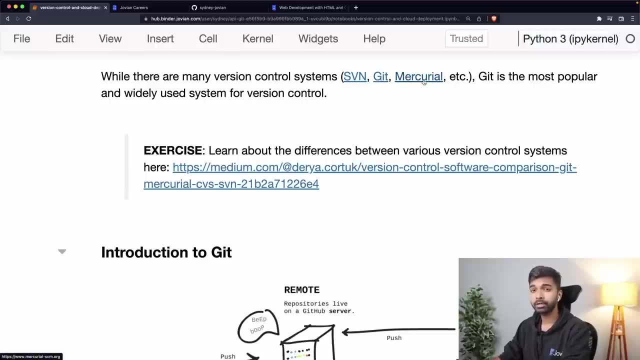 So there are many version control systems. There's one called SVN that was very popular early, early on in the nineties. There is, of course, Git, which we'll talk about today, And there is something called Mercurial. So version control system is any system that allows developers to track various 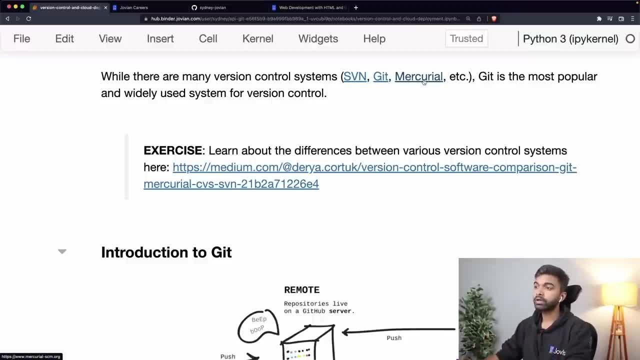 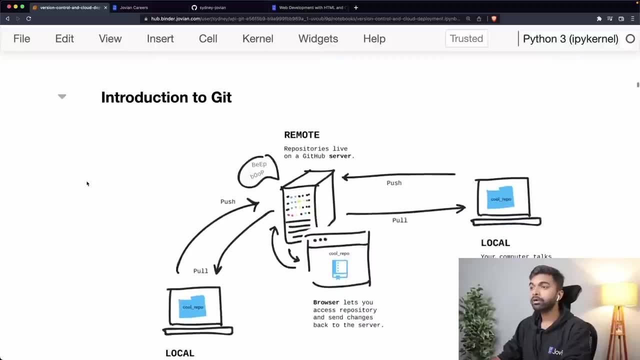 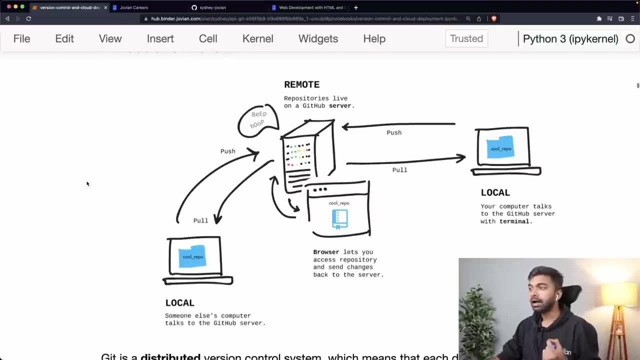 versions, track changes of files or projects. Now you can learn about the various version control systems and the differences between them. I've linked to a site, but we are going to focus on a specific kind of version control system called Git. Now, the key concepts behind Git are that you have typically a remote server. 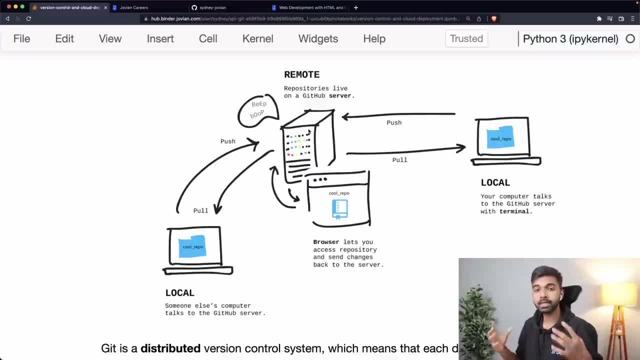 So typically, this remote server could be something that you have set up, Your company has set up, or it could be an online platform like GitHub. So you have a remote server where the ground where the master version or where the main Inversion of your code is stored, and this board is called a repository. 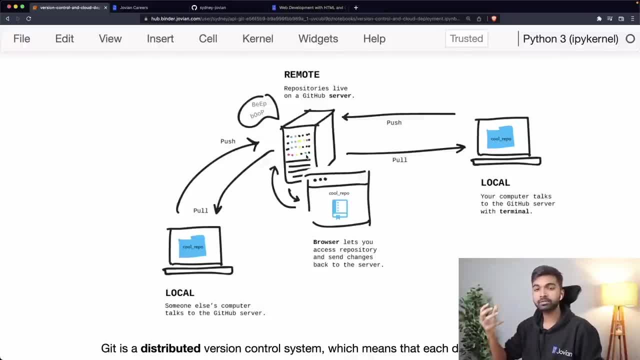 So your code is stored in something called a repository, along with all its previous versions, And then, whenever you, as a developer, want to work on this code, you first have to pull it onto some computer, So it could be a local computer, It could be another cloud computer, and then you make some changes on your computer. 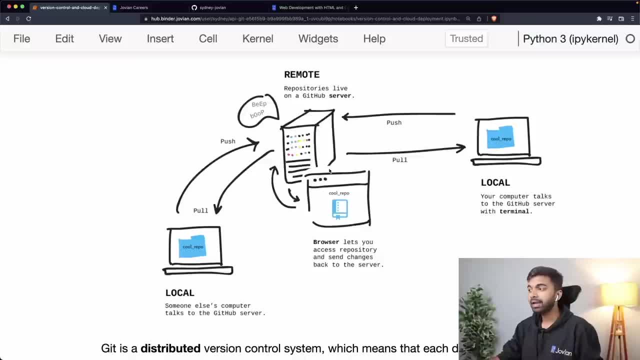 And then you send the changes back to this remote server. and you're not just the only developer. If you want to work on this, there can be other developers who can be doing the same thing. Okay, So Git is this particular kind of version control system where you have now often the 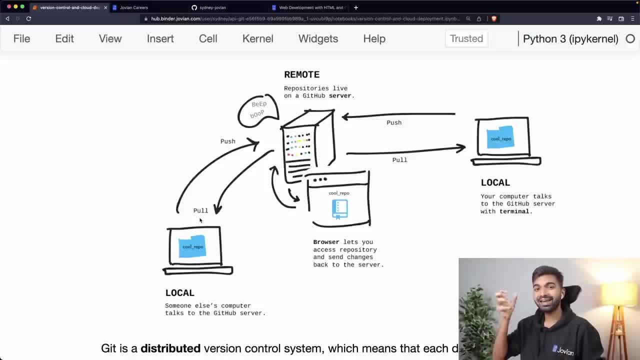 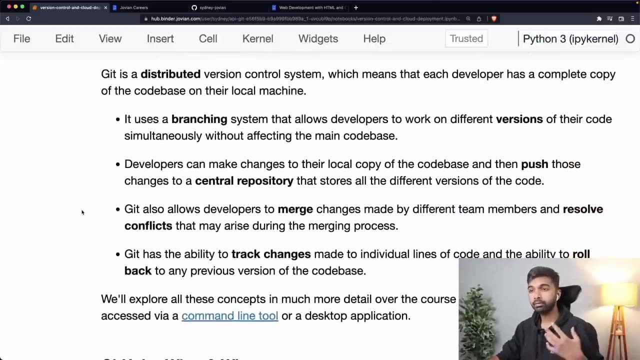 central server which stores the repository of code, and then you take a copy of the code, make some changes and push your changes back to the central server, And that is how people collaborate. Okay, So that is how Git works, And here are a few concepts in Git that we will try and cover today. 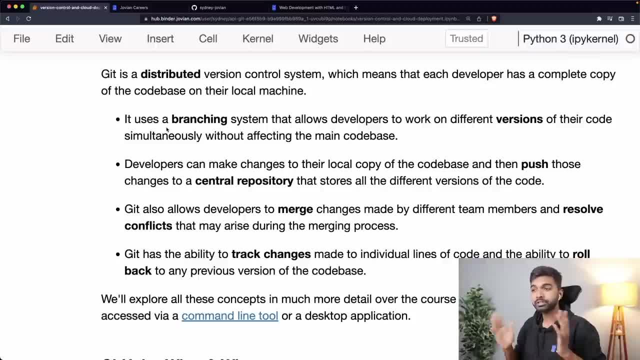 So the first thing in Git is that it has it. It uses something called a branching system that allows developers to work on different versions of their code simultaneously without affecting the main code base. Okay, The second thing is that developers can make changes to their local copy, and then they 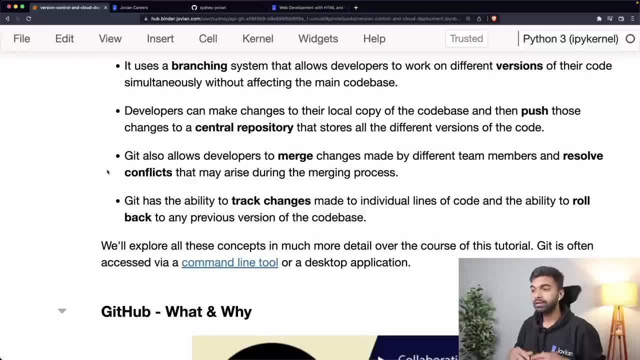 can push those changes to a central repository. Next, suppose two developers are making changes to the same file or the same set of files. Then Git also allows developers to merge their changes, the changes made by different team members, and resolve any conflicts in case both team members are making changes to the same file. 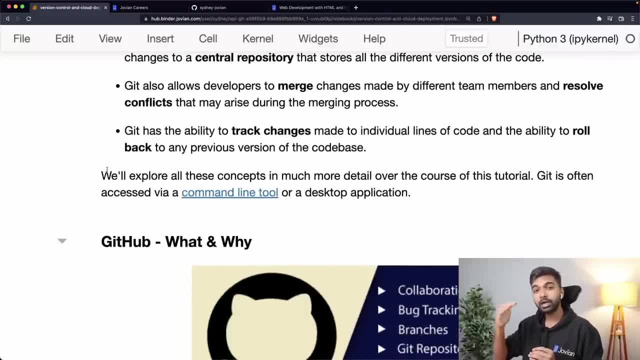 Finally, Git also has the ability to track changes made to individual lines of code. So when you're trying to merge some of your changes back to the cloud repository, you can check what individual lines of code have changed, and you can also roll back to previous versions of the code. 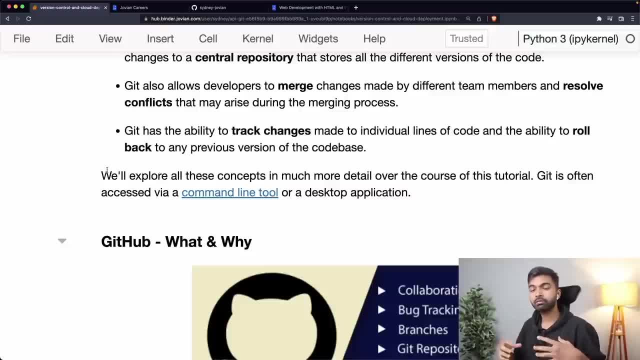 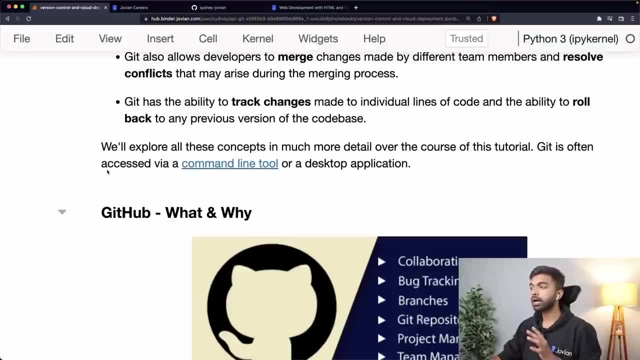 Okay. So it is one of the more sophisticated and one of the most widely used version control systems, And don't worry if these concepts don't make sense Right now. we are going to cover all of this in much more detail over the course of today's tutorial. 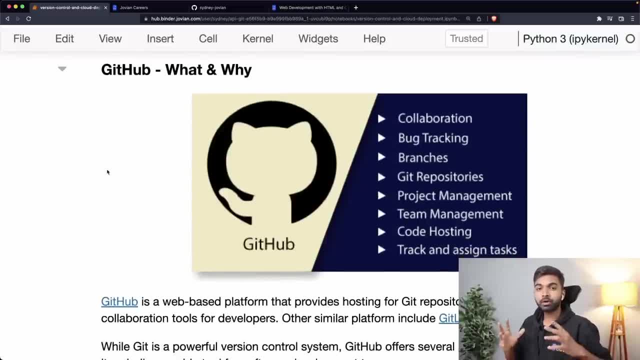 Okay, Next, what is GitHub? So we talked about version control, any system that can be used for tracking changes across files and folders. Git is a particular kind of version control system where there's a central repository and then you can take copies, make. 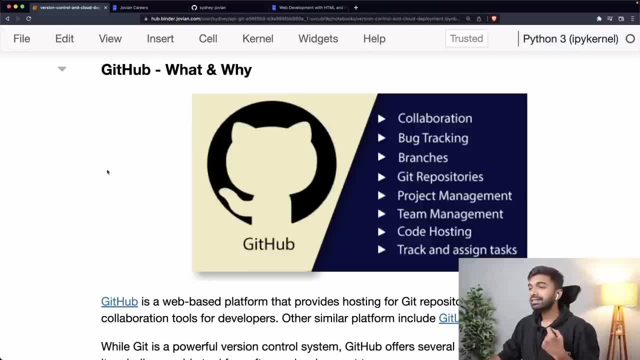 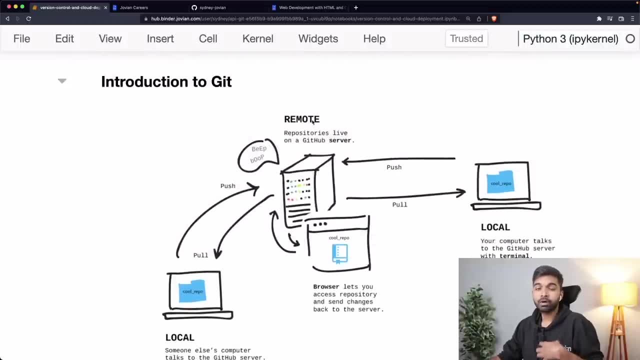 changes and push them back using branches. Then we have something called GitHub. Now, remember, in Git there is the central repository. That can be a repository that you have set up, your company has set up, or you can use one of existing central repositories. 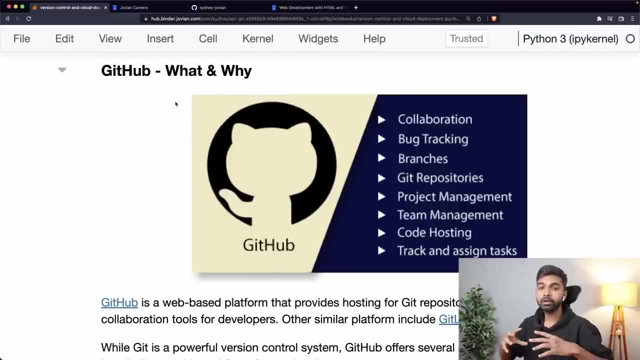 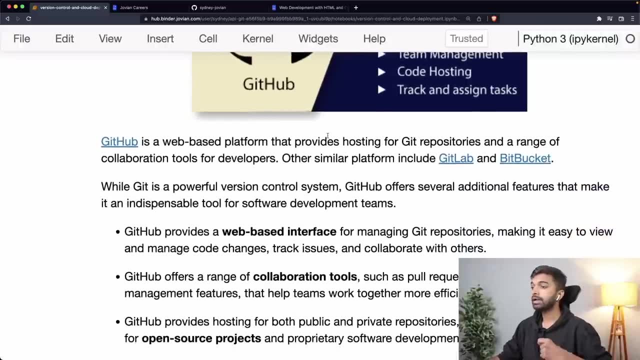 And GitHub is the world's largest central repository for Git-based projects. Okay, So GitHub is a web-based platform that provides hosting for Git repositories And it provides a range of collaboration tools on top of that hosting for developers. Other similar platforms are GitLab and Bitbucket. 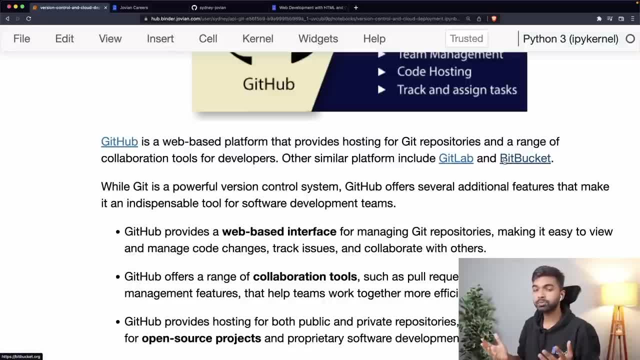 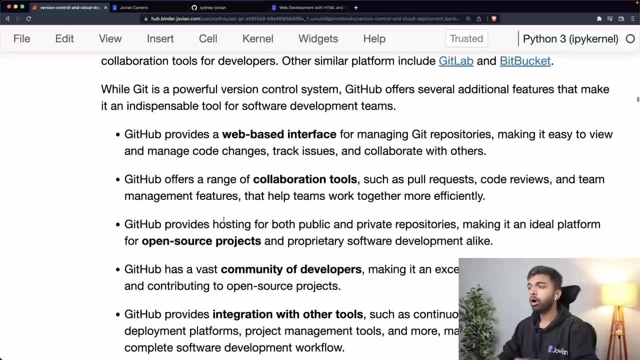 So you can use any of these. all of them have free plans, But GitHub is the most popular one. It has tens of millions of people using it, So you should probably start with GitHub Now. on top of Git, GitHub offers several additional features. 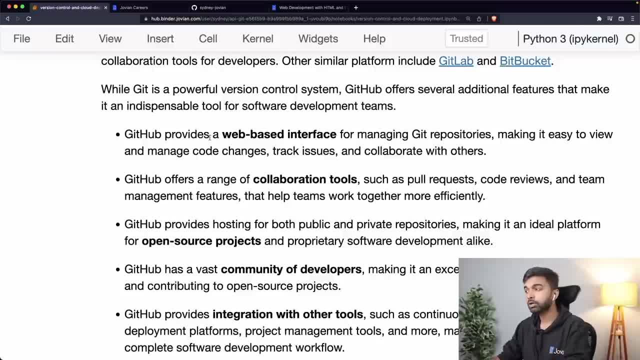 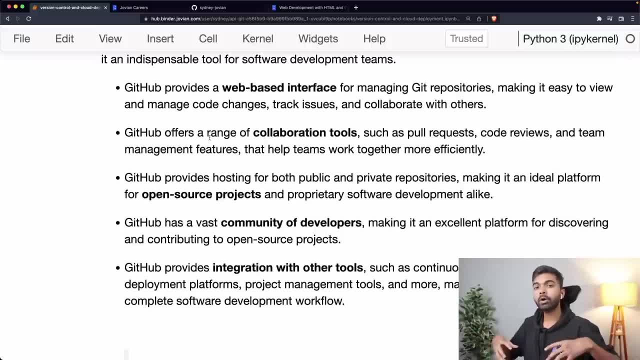 The first thing it gives you is a web-based interface for managing Git repositories, making it easy to view and manage code. It also offers a wide range of collaboration tools on top of Git- things like pull requests, code reviews and team management features. 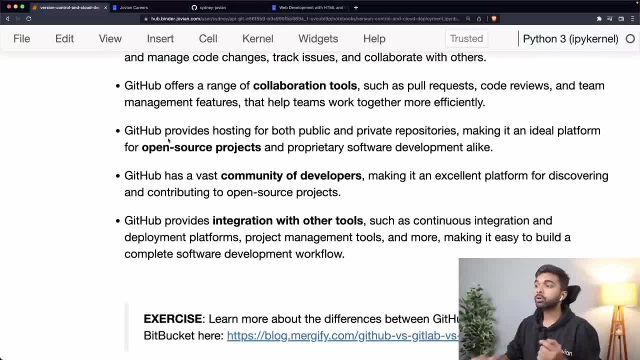 Again, we'll touch on these. And finally, GitHub. It also provides hosting for open source projects. So most software that you use on the internet is built using open source projects, And these open source projects are typically hosted on GitHub. So GitHub is a great place for you to discover open source projects and even contribute to open source projects. 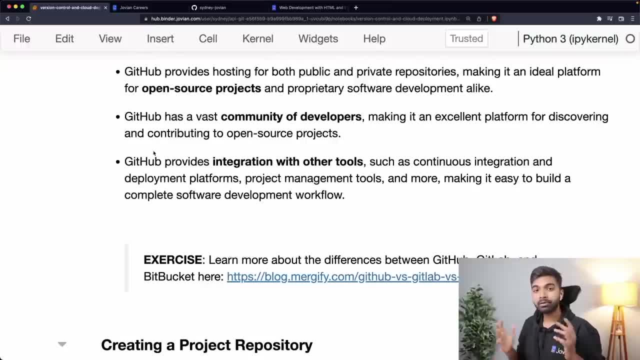 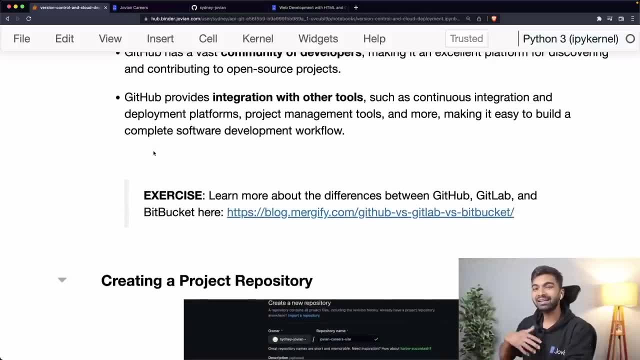 And it has a vast community of developers where you can interact with others, and you can interact with developers of open source projects and make your own contributions. Finally, GitHub also provides integrations with other tools, Specifically around diplogs, Deployment, project management, et cetera, to make it a complete software development workflow. 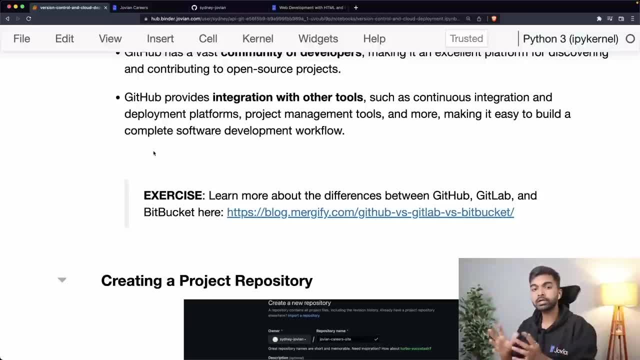 Okay So GitHub is a hosting platform for Git and it offers a lot of additional features on top of Git. Okay, So I hope that clarifies the difference between Git version control and GitHub. They are like layers. Version control is a basic kind of a system. 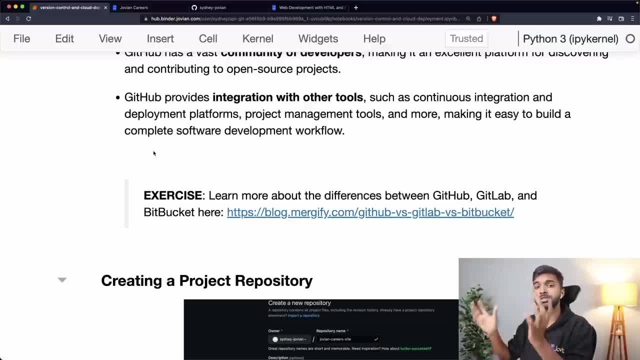 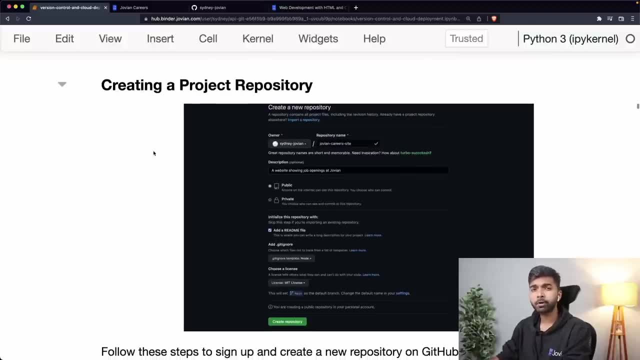 Git is a specific kind of version control system and GitHub is a hosting platform for Git repositories with some additional features. So let's start by first creating a repository for our project. So projects on GitHub are known as repositories, So we'll go ahead and create a repository. 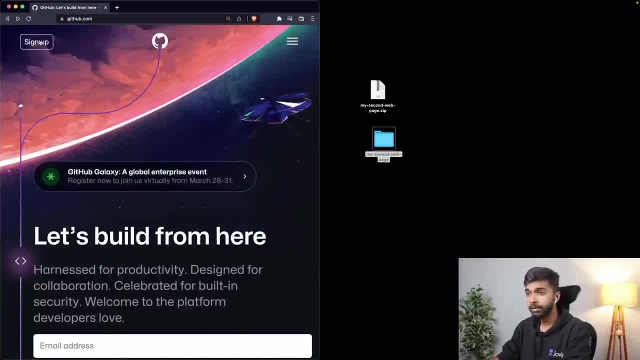 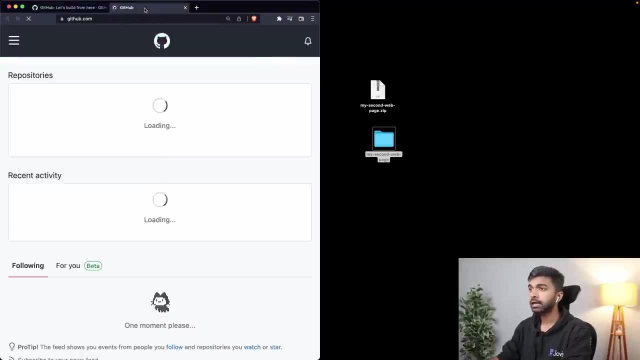 So the first thing you might need to do is go to githubcom and sign up, if you're not signed up already. In my case, I have already signed up, so I'm simply going to sign in. So I'm just going to click sign in and that is going to sign me in to GitHub. 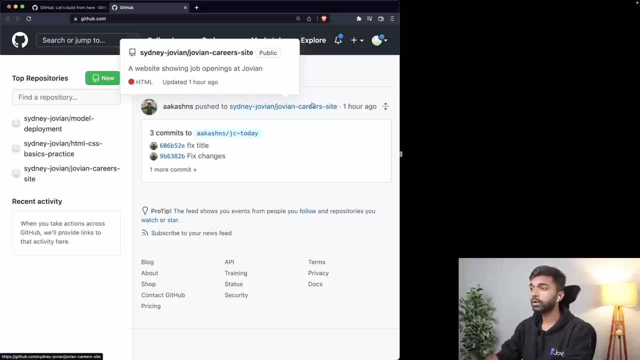 All right. So once you sign in, this is what your dashboard looks like, And on your dashboard, the first thing you want to do- at least when you've created your account for the first time- is to click the new button to create a new repository or a new project. 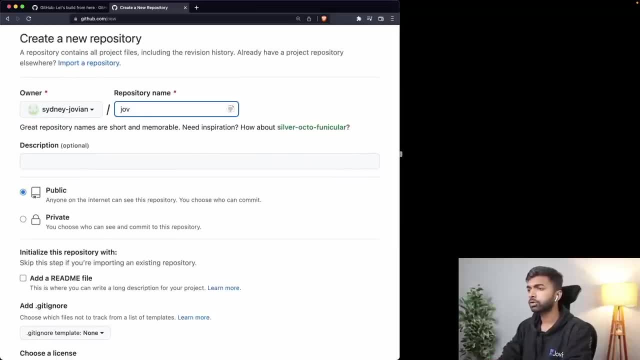 So let's create a new repository- We are going to call it Jovian careers site- live, because I'm doing this live- and let's add a description for this repository. So a website to show job applications at Jovian, Our job openings at Jovian, and accept applications. 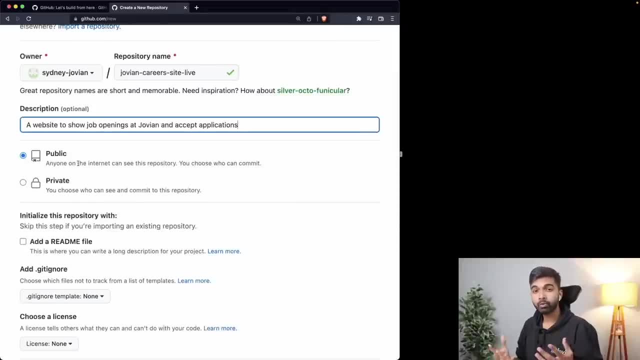 Next, you can choose whether to make this repository public, which is open source for the rest of the world to see and build upon, or you can make it private. Now, you can make it public and people can see the code, but they cannot make changes to your repository. 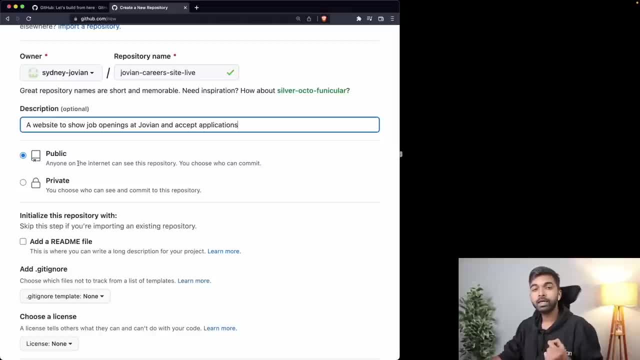 You still control who can make changes. but if you make it private, only you will be able to see it, And if you add Collaborators, only they will be able to see it, And you can also choose which of those collaborators can actually make changes to the repository. 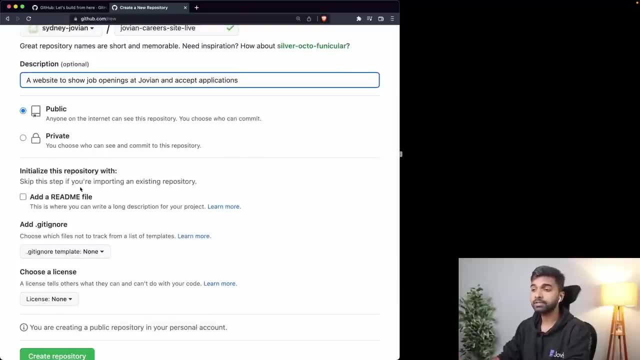 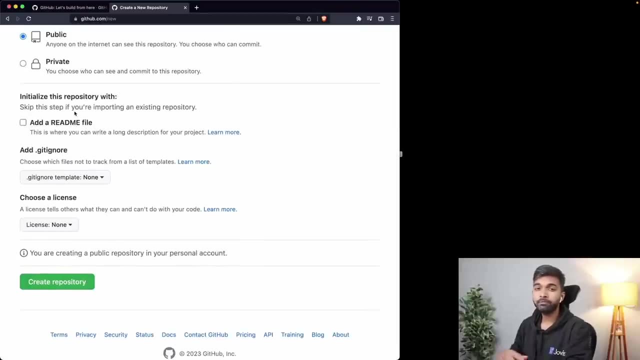 So far. now I'm just going to make it public so that you can actually see the code by the end of this lesson yourself. Next, you have a few initialization steps. So if you are creating a repository on GitHub and you plan to develop from this repository, then you should initialize it with a readme file and some of these other things. 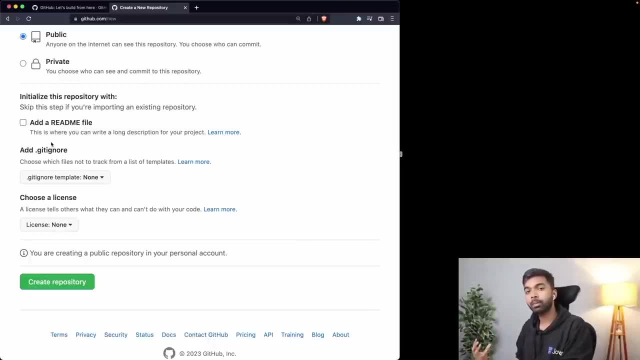 On the other hand, if you already have a repository on your computer, You just want to upload it to GitHub, Then you can skip these initialization steps. Okay, In my case, I'm just going to select this initialization step. add a readme file. 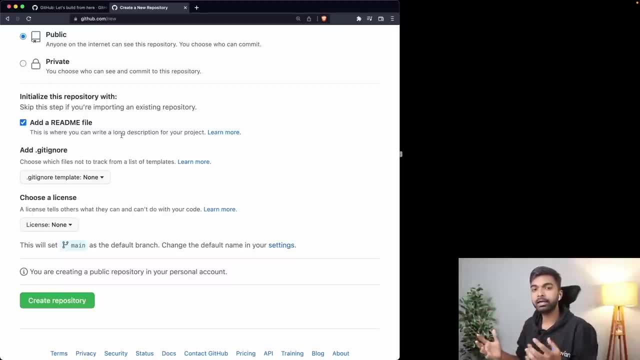 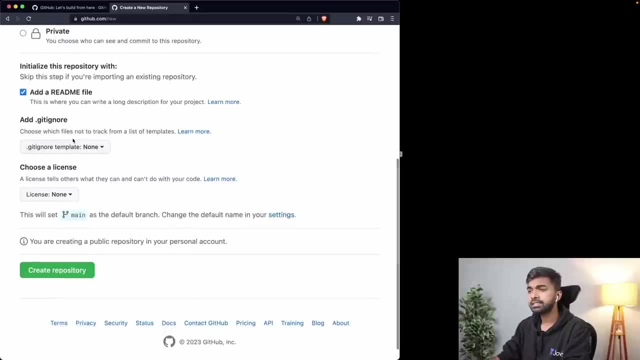 What that's going to do is just create a file called readmemd wherein I can put in some documentation about my project, So I'm going to keep that. And then there is something called a gitignore file that gets added So often when you are creating a git repository. there are certain temporary files that can get created as you're executing your code. 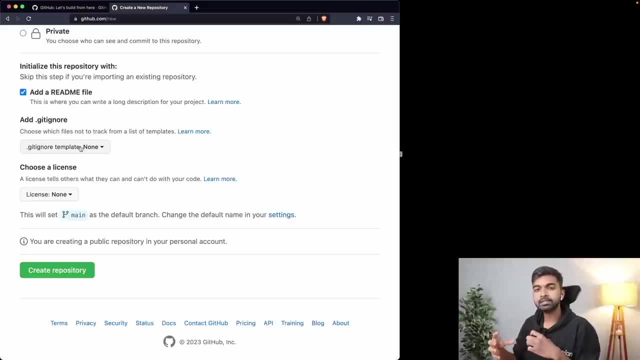 Okay, And you may not want to put those temporary files or compiled files into your git repository, So that's where a gitignore file comes in. Don't worry about this. We'll touch on this later, but for now, because we are going to create a JavaScript and HTML and CSS project, 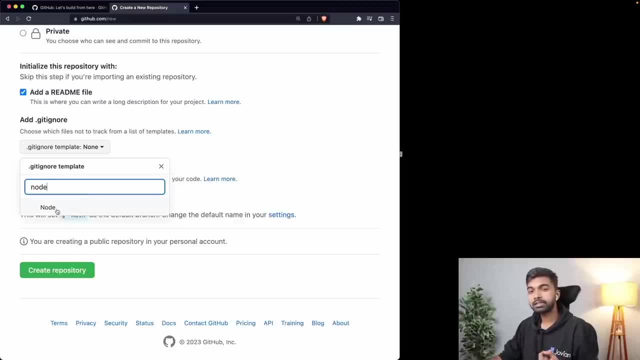 So the top, the gitignore template that you can select, is node. So node simply stands for nodejs, which is a tool used to run JavaScript and HTML and CSS based projects Locally on people's computers. So you can just select the gitignore template: node. 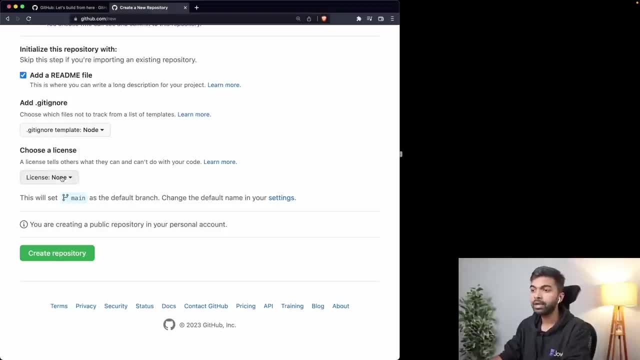 And if it doesn't make sense, don't worry, it's not important right now. And finally, you can also select a license. So when you put up any code on the internet, specifically on GitHub, you can inform people what you, what they're allowed to do with the code. 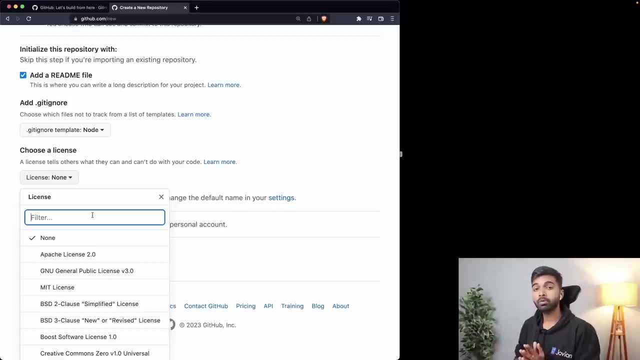 Are they allowed to build on top of the code? Are they allowed to use the code for academic purposes? Are they allowed to use the code for commercial purposes? You can specify All of that, And one of the most common licenses is the MIT license, which basically allows the user of your code to do anything they want to do with the code whatsoever, without any warranties. 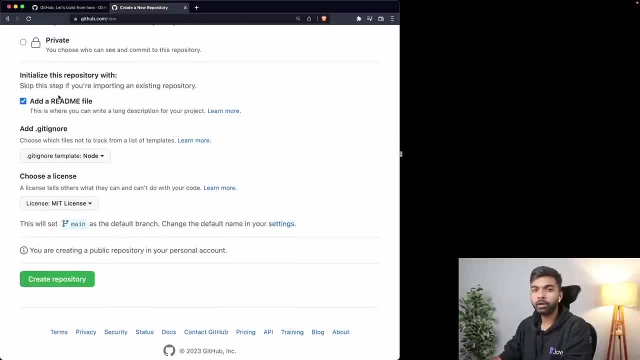 Okay, So that is just a common template. So what you'll often do when you create a new GitHub project is you'll add a readme file. You will select a gitignore template for JavaScript or HTML CSS projects- These- this is typically node, but let's say, if you were doing a Python or a data science project, you could select Python. 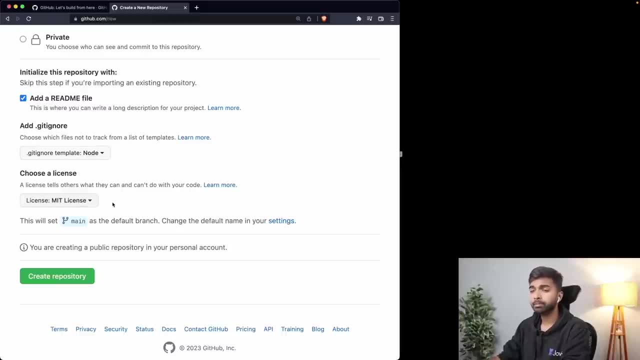 And so, And you will also select a license. in many cases, MIT license should suffice, And you can learn more about all of these- the readme file, the gitignore and the license- by checking out these links. Okay, Now, finally, as I said, git has a concept of branches. 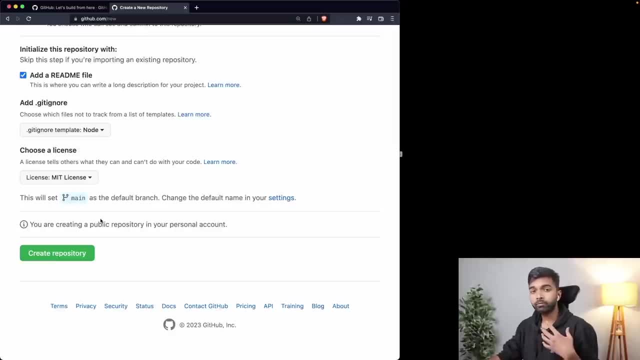 So the first thing you have to do is, when a git GitHub repository gets created, it has a default branch, and the default branch is often called the main branch- Okay, The main branches where the main version of your code Code lives. but you can then create multiple branches as you're working on specific features, and then you can um bring those code from those branches back into the main branch. 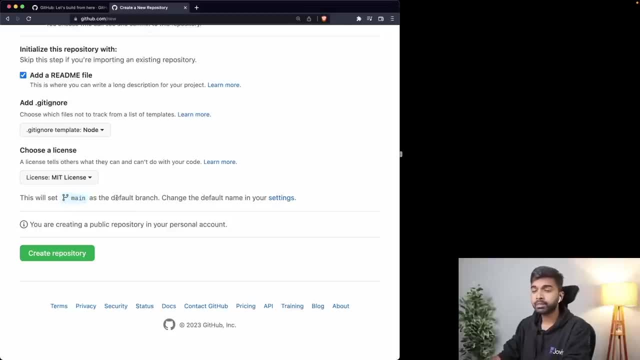 Now, for now, uh, we will go ahead with main as a default branch. but know that sometimes in some older repositories, the, the default branch name was called master M A S T E R, but the new convention is to call the uh default branch main. 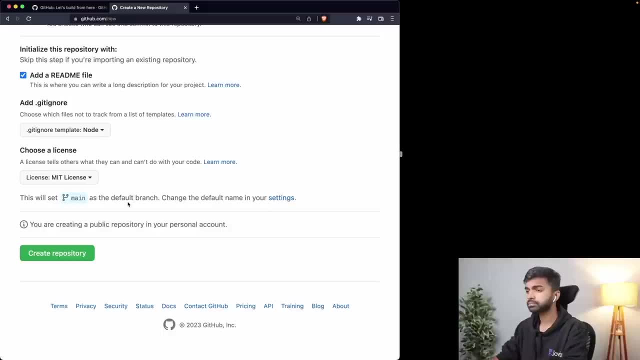 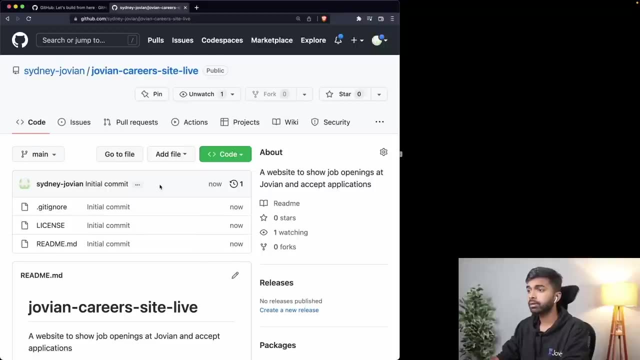 So that's what we'll go ahead with, Okay, Okay, So let's hit create repository. And now our GitHub repository is created. Perfect, So you can see, now you have this fairly complicated looking interface. You have a nav bar here, then you have a bunch of buttons and you have a bunch of tabs and you have again some options, et cetera. 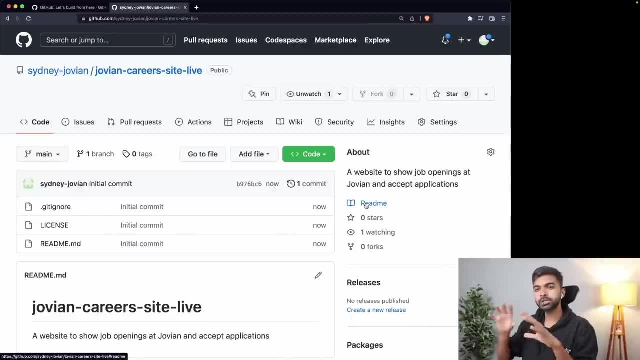 So I know it looks complicated, but we will touch on all- almost all- of these tabs over the course of the next several lessons and over the course of the program, But for now, what I want you to pay attention to is this area. 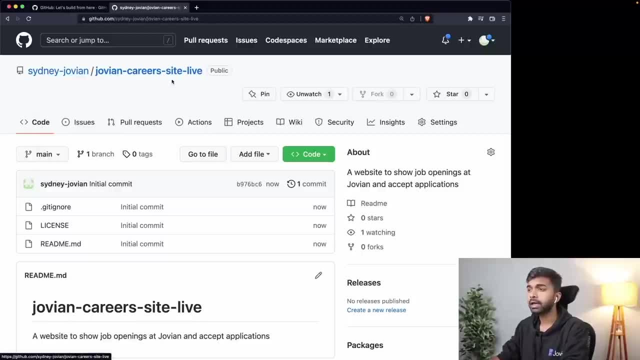 So here Is your username. You will see your username here, and next to your username you will see the name of the project. So the name of the project is Jovian career site life. Typically these are all lowercase And typically these are all separated by hyphens. 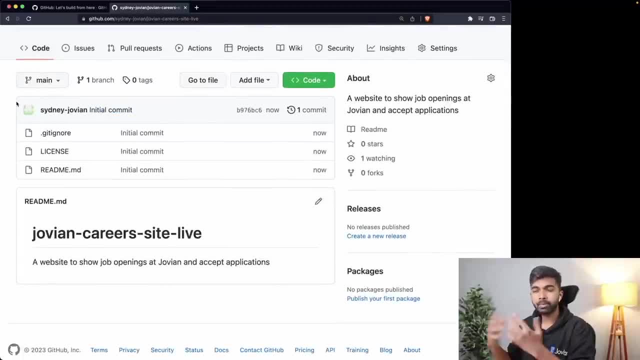 And then in the core tab, you're going to see that in the main branch, which is the only branch we have right now, we have three files. So our repository has been initialized. You can see that there's an initial commit. Uh, we'll talk about comments as well. 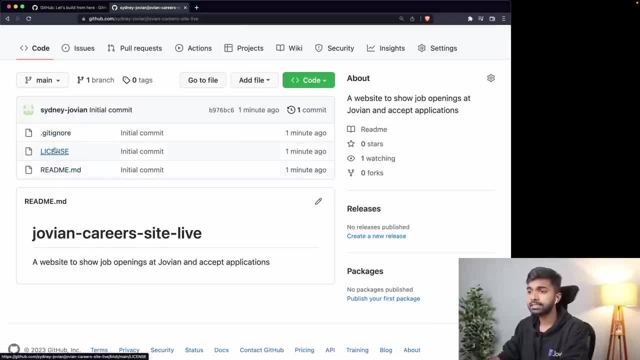 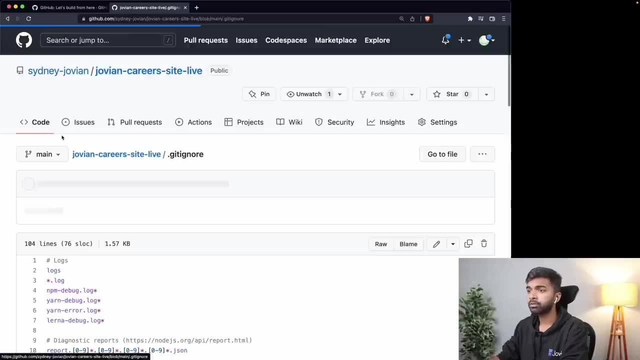 One minute ago with three files. One is a read me file, One is a license file, One is a getting no file, and you can open up this license file and you can see what it contains. Similarly, you can open up this get ignore file and you can see what it contains. 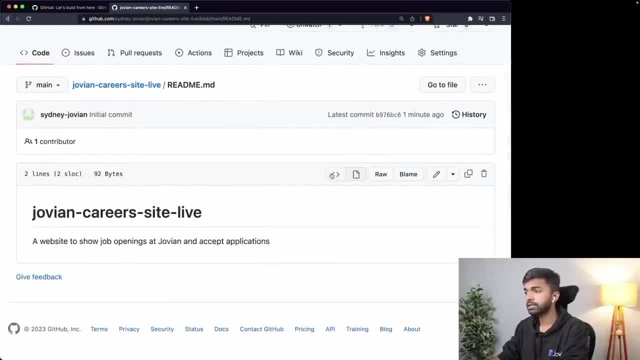 And you can open up this readmemd file and you can see what it contains. So, again, this is all created using Markdown, which is a fancy way of writing text. So there are three files in our repository and, at the moment, our GitHub project. 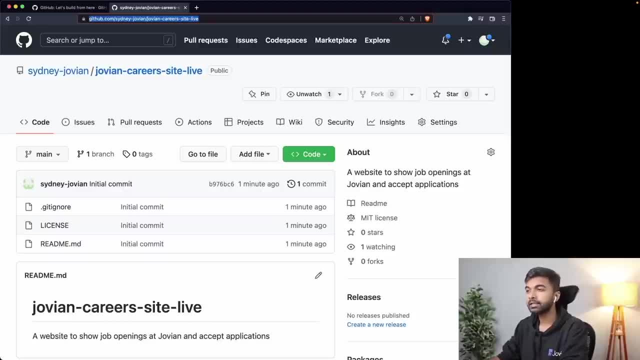 Our repository has been created, so we can already go ahead and share this with other people. Let's say, we want to share our code with other people. We can take this link and share it with them, but of course we don't have any code here right now. 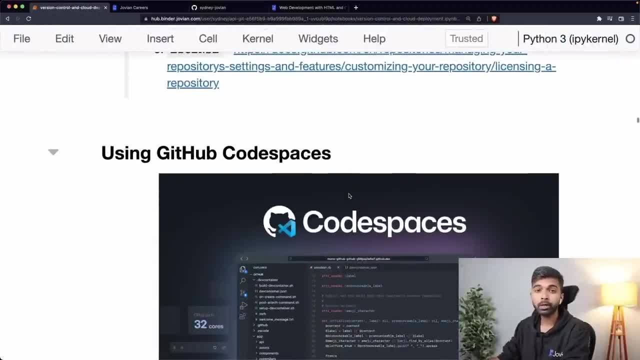 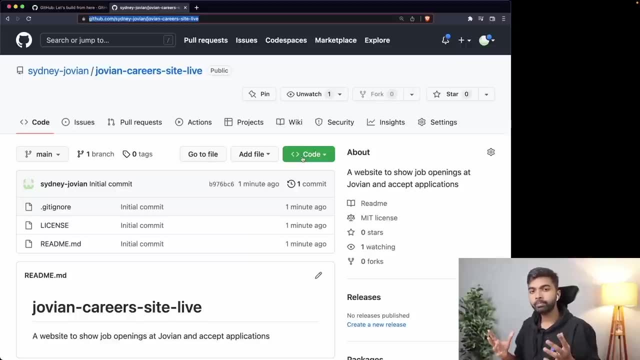 So the next thing we're going to do is actually import our code into this repository. Now there are two things we can do. We can actually start writing writing some code, or we can start importing some existing code that we already have. in both cases, 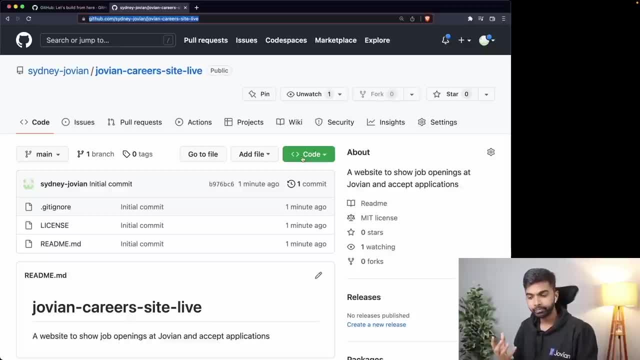 We need to open up this Git repository- Git repository- in a code editor. Now you can download this Git repository to your computer and then open it up in VS code or any other code editor, or you can also use some online platforms for developing on this GitHub repository. 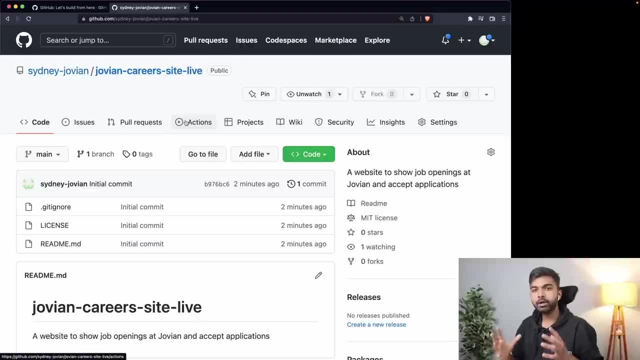 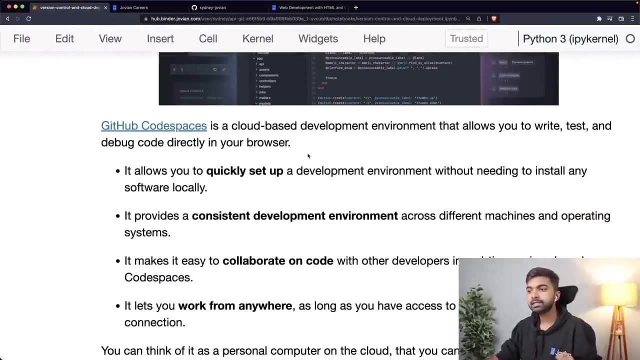 Specifically, GitHub provides something called GitHub code spaces, which you can think of as your own personal computer, attached to this GitHub project or repository, but living on the cloud, All right. So GitHub code spaces is a cloud-based development environment that allows you to write, test and debug your code directly in the browser. 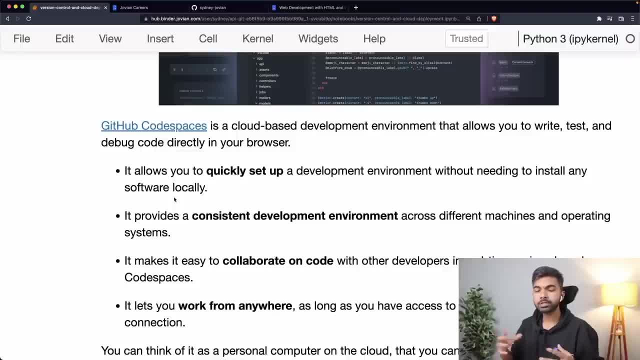 So it allows you to quickly set up a development environment without needing to install any software locally. It provides a consistent development environment across different machines because you're writing all your code in the browser and the browser is connected to some machine on the cloud where all of the dependencies are already installed. 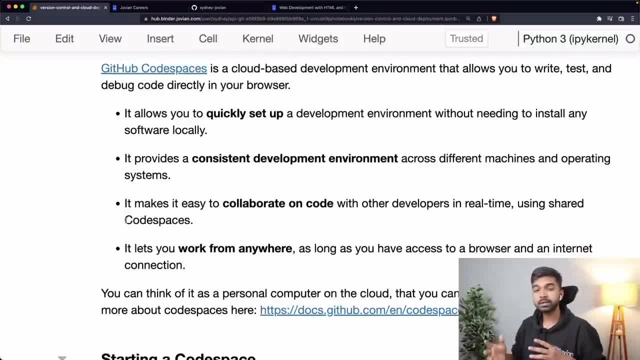 It also makes it very easy to collaborate on code with other developers Because you can have real time shared code spaces. So if you're writing code within a code space, you can create a shareable link, invite somebody else to come and collaborate with you live. 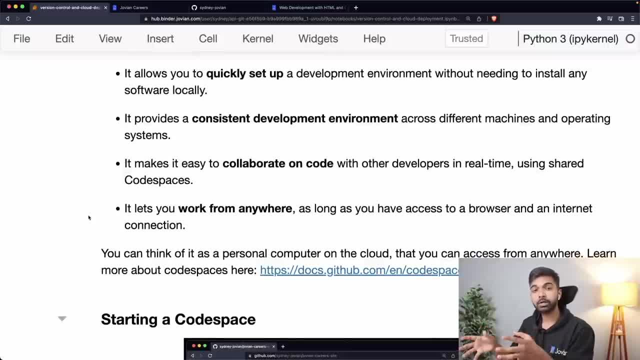 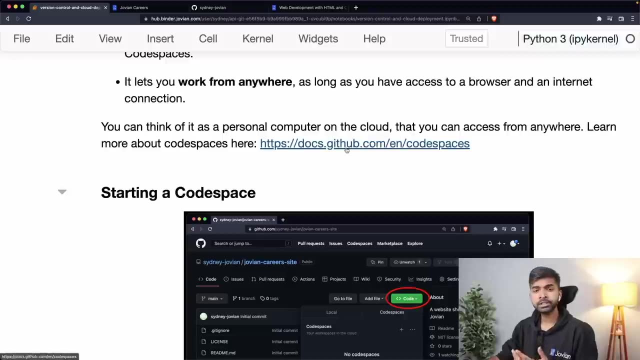 And it lets you work from anywhere, So you don't have to work from a particular computer. You can just open up your GitHub repository and launch a GitHub code space online and start typing code into it. Okay, So you can think of it as a personal computer on the cloud that you can access from anywhere and you can check out GitHub's documentation for. 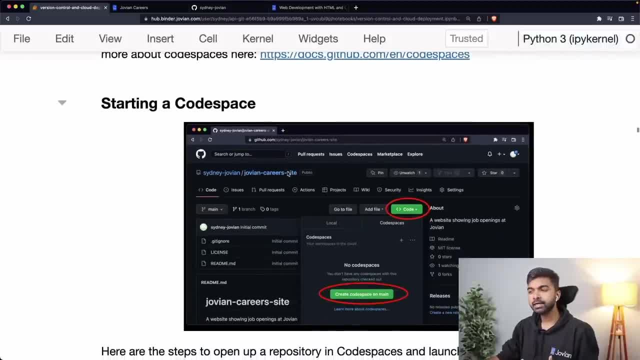 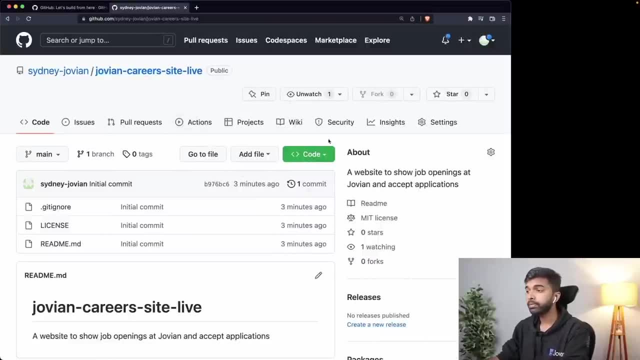 Setting up code spaces. but starting a code space is really simple. What you do is you go to your repository folder and you go to your repository on GitHub and you click this code button here and you have two options. You have local and you have code spaces and here you can click create code space on main. 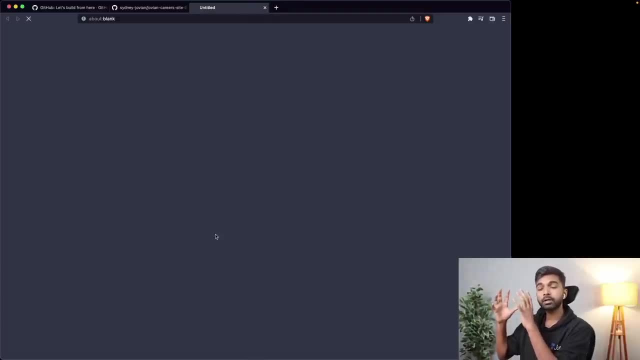 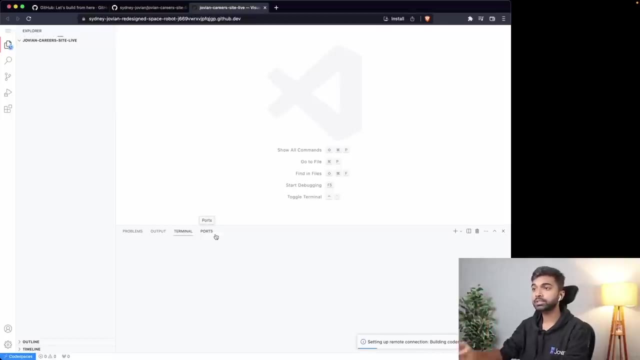 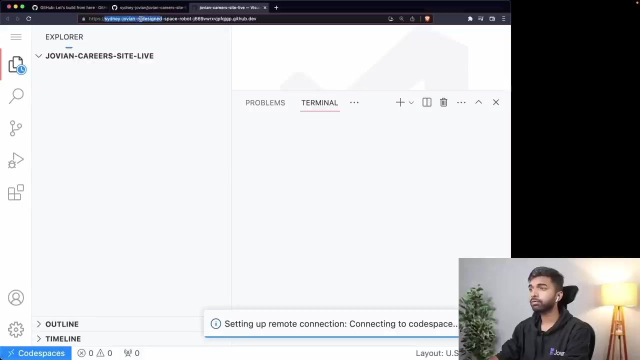 So what this is going to do is this is going to set up a computer for you on the cloud and it is going to associate that computer with This GitHub repository. So you can see here, if I zoom in a little bit, it has set up this cloud based computer for me and it has opened up visual studio code on that computer. 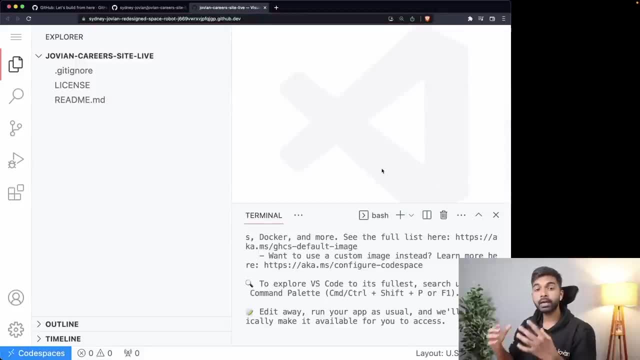 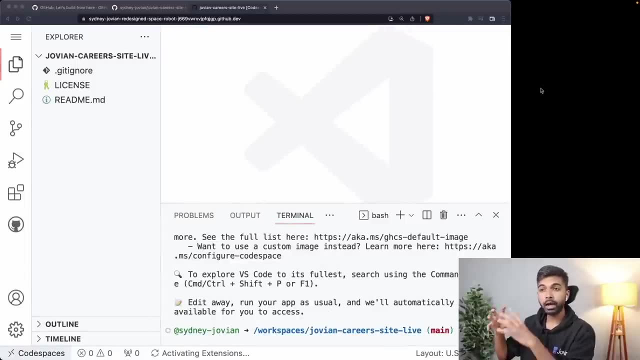 And it has given me a browser based interface to connect with visual studio code on that computer. So there's a lot going on here. So instead of opening visual studio code on our own computer, we have opened up visual studio code on a GitHub code space, which is a. 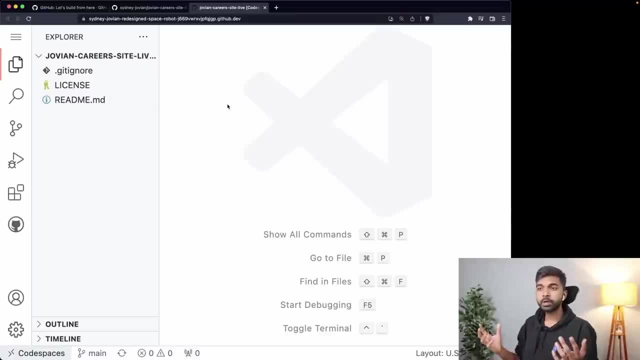 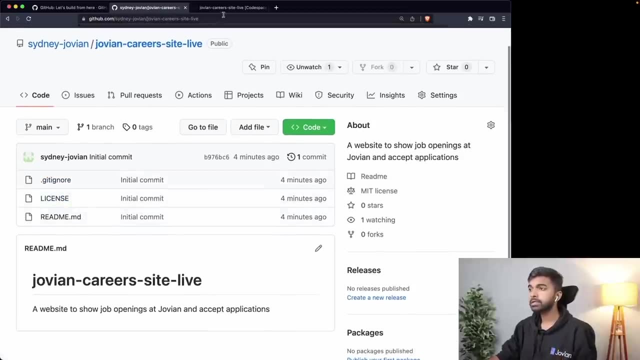 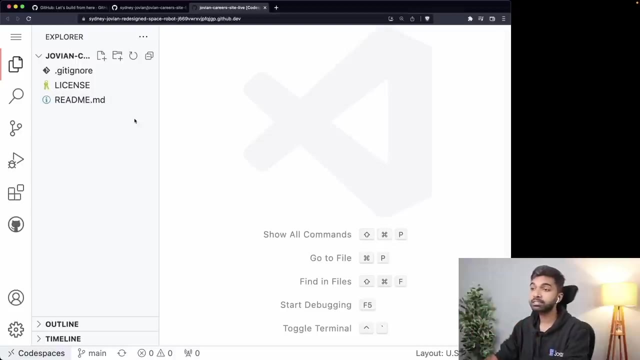 Computer running somewhere on the cloud, All right. So this is what it looks like. Remember we on our GitHub repository, we had these three files: get, ignore, license and read me, dot MD. So if you come here now, you can see that we have the same GitHub repository now open for editing in this code space accessible via these, via this browser based visual studio code interface. 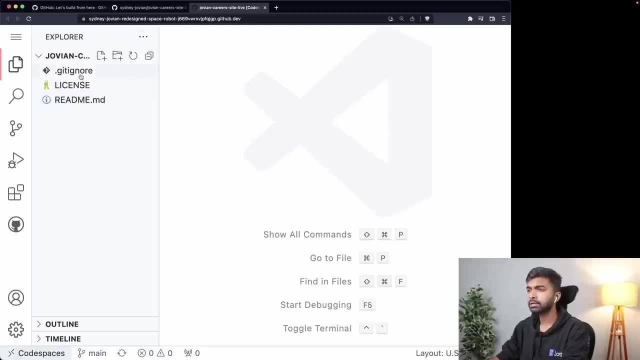 Okay, So within the browser we have visual studio code and I can open get ignore and I can make some changes here. and I can open this license file and I can make some changes here And similarly, I can open this read me file. 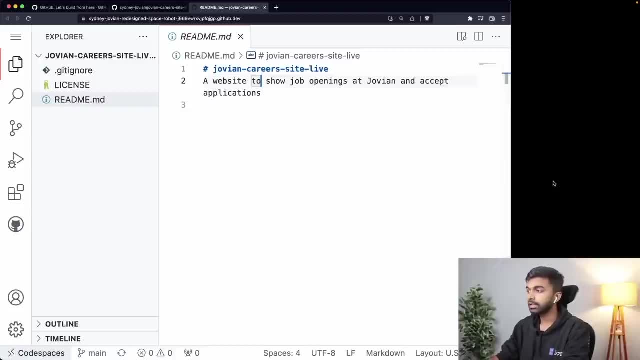 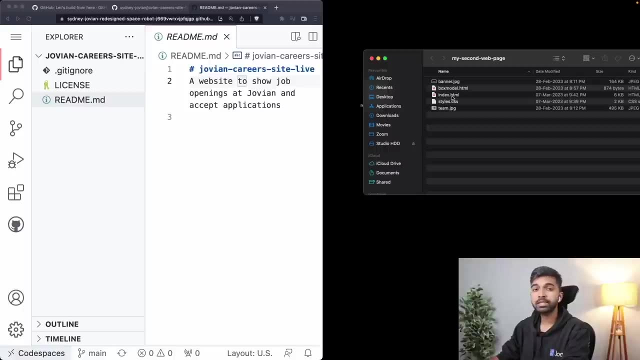 And I can make some changes here. Okay, But what we want is to actually put in the code that we already have from our previous tutorial, which is the index, or HTML, styles, dot, CSS and a couple of other files. So here's what we'll do. 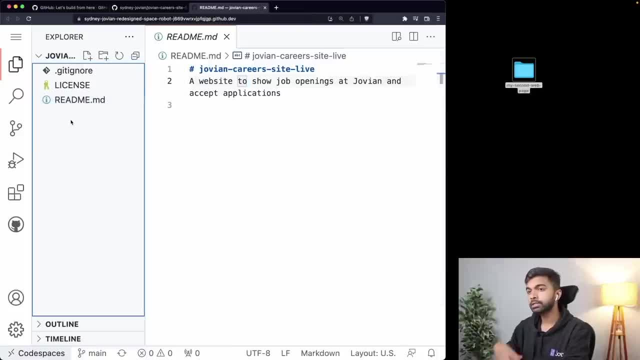 As you work on more complex projects it is going to, it's it'll be a good idea for you to separate some of these configuration related files, like get, ignore, license, et cetera, with your actual source code. So what I'm going to do is create a folder. 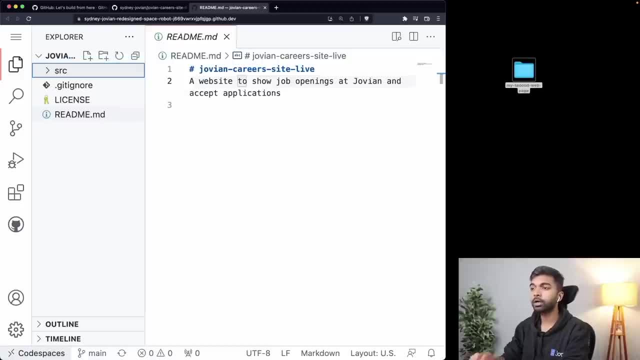 Here. So I'm going to right click and select new folder and I'm going to create a new folder called SRC. So now I have created a new folder called SRC and into this folder Now I can add an index or HTML file. 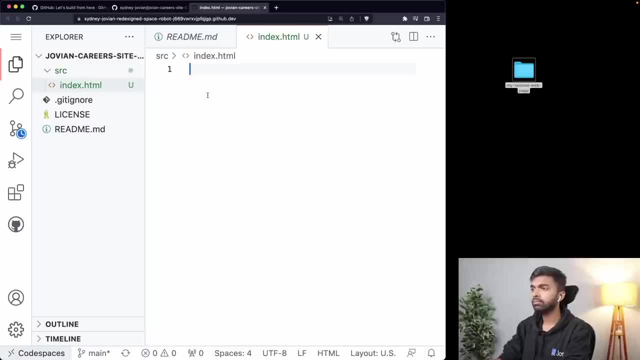 So I can say index dot HTML, and now I can maybe put in some HTML code here and maybe I can start writing things and so on. but I already have a bunch of these files, So I can just upload these files. So let me delete this file once. 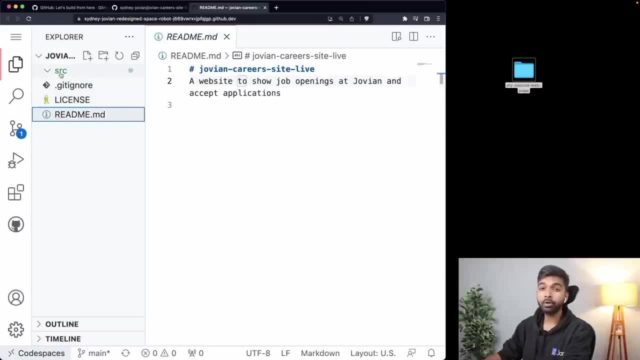 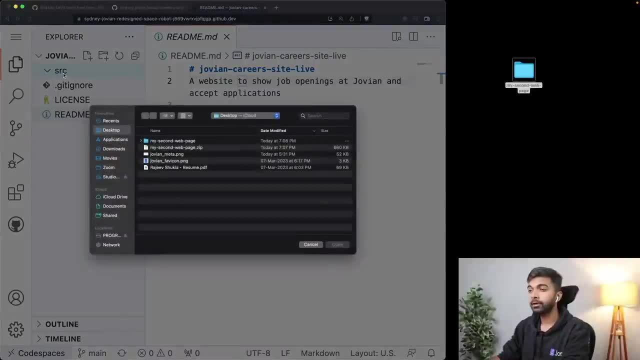 Let me just delete this file index or HTML, And let me upload these files from my computer onto this remote machine. So I'm going to say upload, I right clicked on SRC and I'm clicking upload and now I'm going to open up the folder- my second webpage- and now I'm going to select the files that I want to upload. 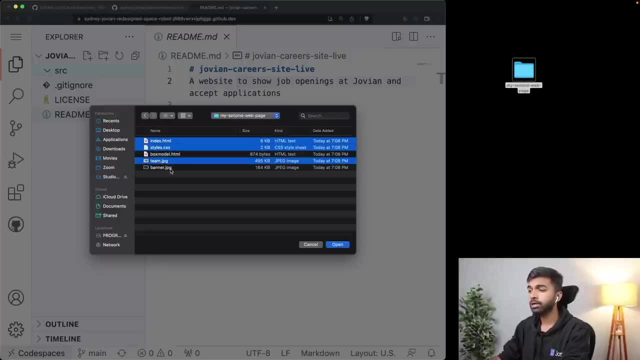 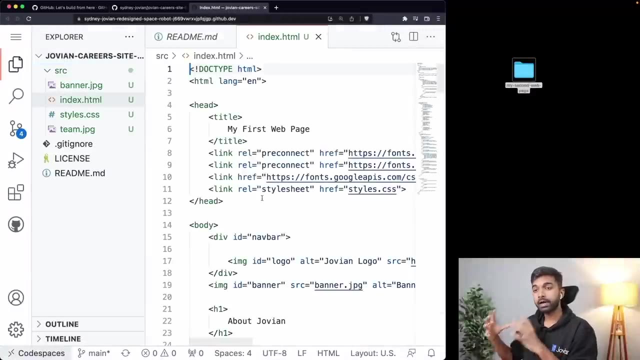 So I want index or HTML, I want styles- dot CSS, I want team dot JPG and banner dot JPG, And I'm going to click open, All right. So now all the files from my computer I've been Taken and uploaded into this cloud code space, this cloud machine, which I'm accessing using VS code from the browser. 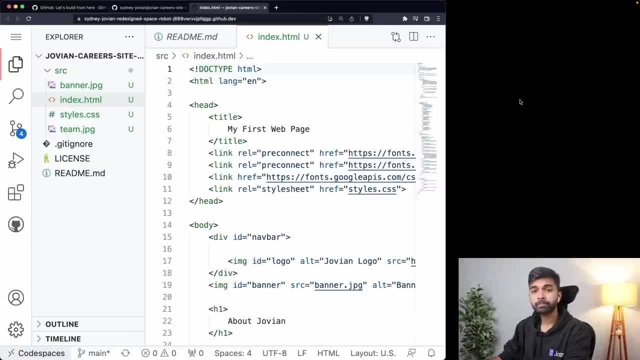 Okay, Now I can, and now we can actually go ahead and delete this folder entirely. I don't need it, but all of this code is still going to be here for me, Okay, So remember, we had this Jovian career site that we built the last time, and this was built using this index or HTML file. 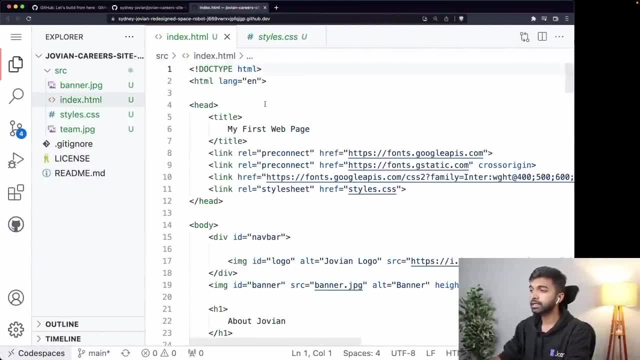 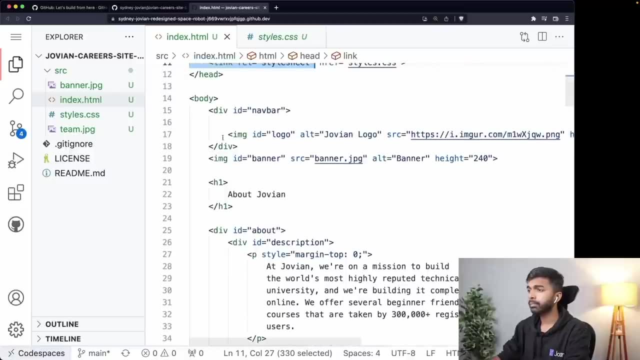 Let us, Yeah, So let us look at this, This index or HTML file. it obviously it has a head section, but it has a title and it has a bunch of fonts that are included. Then it has a body section, which contains a nav bar, which contains a banner, and it contains this heading. 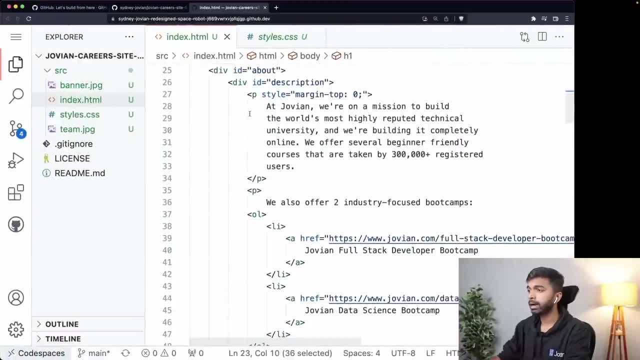 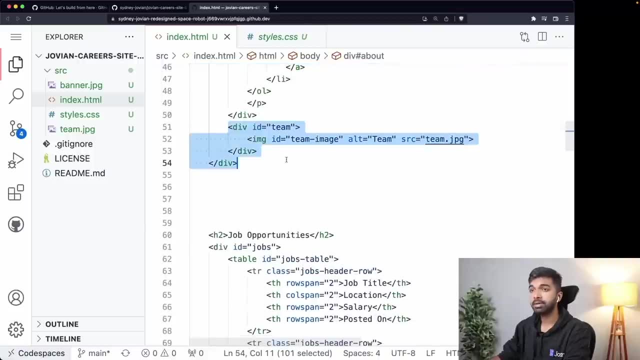 So we have a nav bar banner heading, Then we have this about description section where we have some information about Jovian and we have links to the two programs, And then we have this team image over here and then we have a list of job opportunities, which is a table. 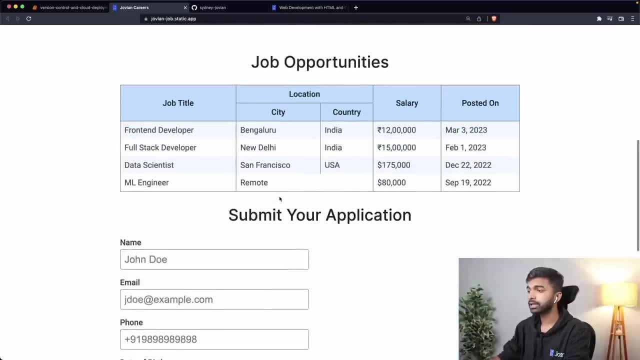 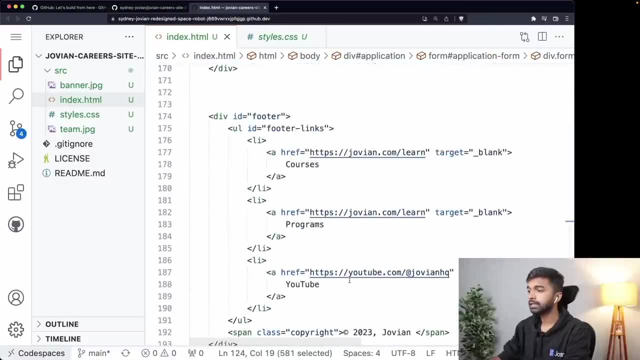 So that is the Job opportunities table that you can see here, And finally, below this, we have a form. The form contains a bunch of form inputs, and then there is a footer below the form, which is what you see here as well. 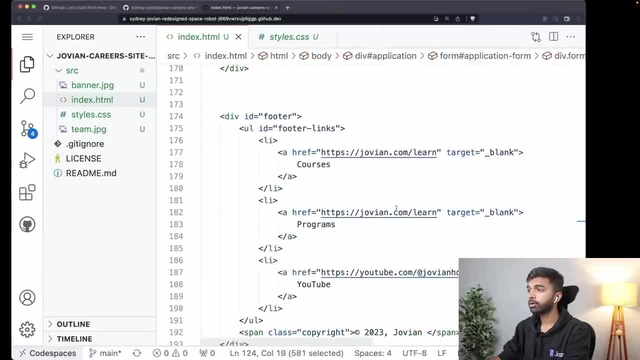 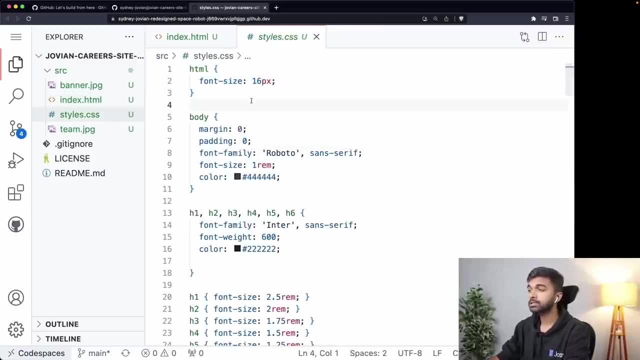 So there is a form and then there is a footer below the form, right at the bottom. Of course, these HTML elements are styled using CSS, So we've set a base font size on the HTML and then we've set some body fonts and we've set some header fonts as well. 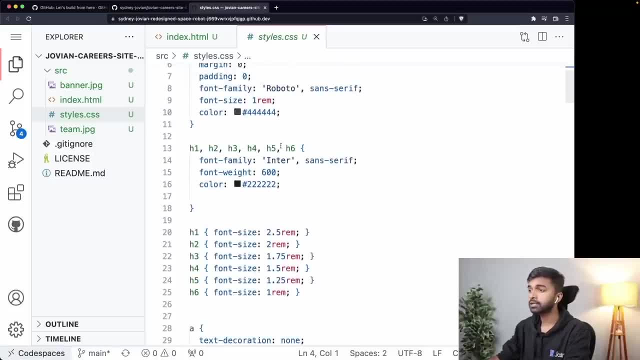 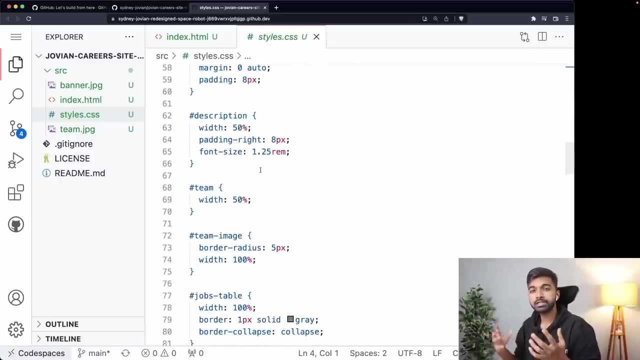 We've also set specific sizes for the headers. We've set specific colors for headers and for body. We've also set a bunch of other colors, and then we've set a bunch of other CSS styles to make our page look as we want it to look. 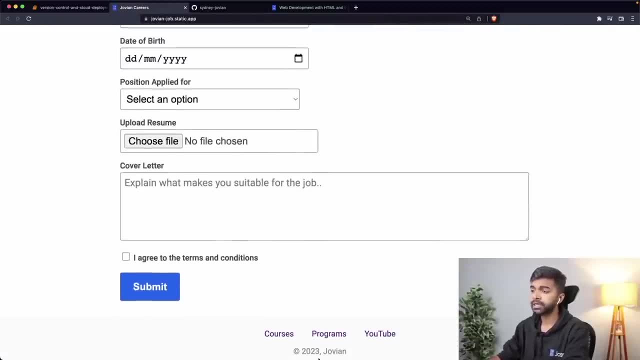 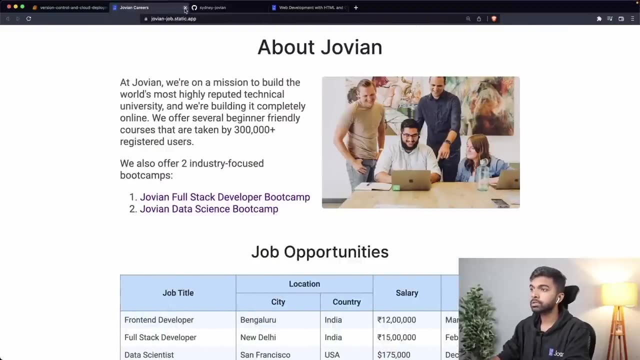 And we have sets and styles for the table, We have set some styles for the form and we've set some styles for the footer and for the button. Okay, So that is what our code looks like right now. So for now, I'm going to close this deployed website, and now let's try and figure out how can we actually preview this? 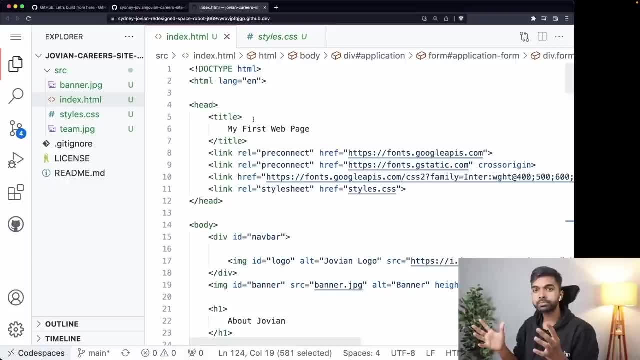 Okay, So now we have some code, Okay, Okay, So we have some code already on this code space, but this code is no longer on our computer. This is on the remote machine, So there's no place where I can double click and open it in a browser and preview it. 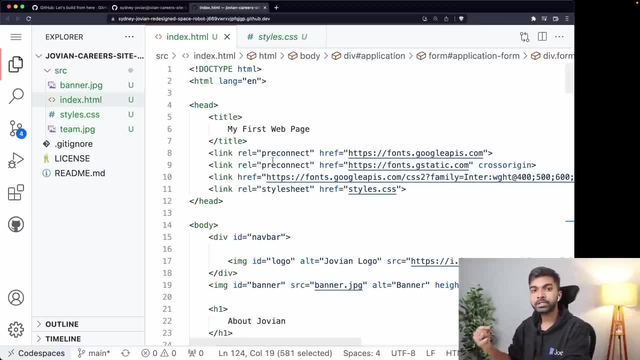 So there is an extension or a plugin that we can install into VS code for previewing these files. All right, So this is one of the nice things about VS code: that, depending on which language or which kind of project you're building, you can install some plugins to ease your development. 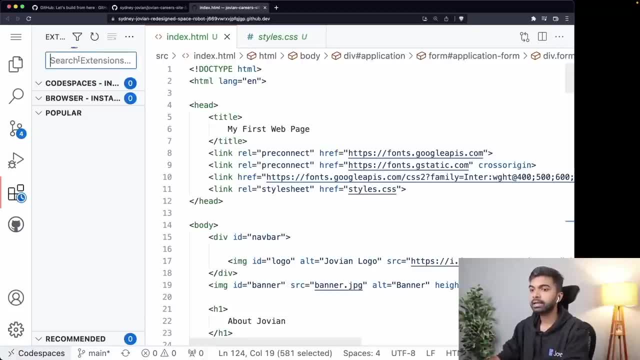 So I'm going to go click on extensions and then here I am going to search for live server. Okay, So just search for live server. L I V E S E R V? E? R. It is created by this person called Ritvik Dey, and you'll know because it has 32 million downloads. 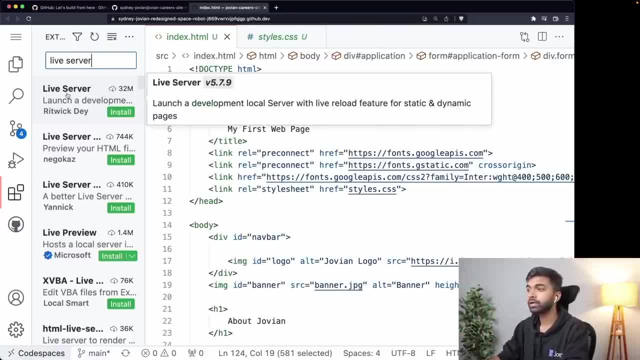 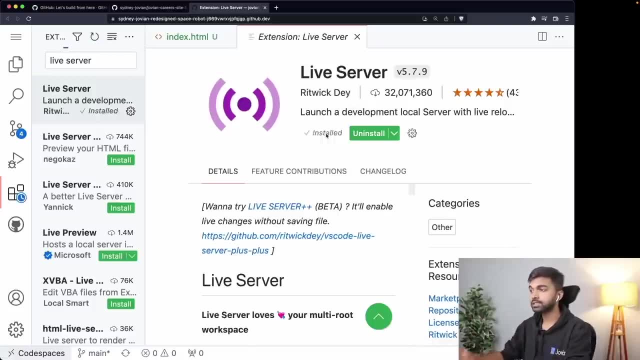 So that is how many people actually use VS code and also use this extension, And I'm going to click install in code space and that is going to install this plugin into my code space. Now, once this plugin is installed into the code space, I can click on install. 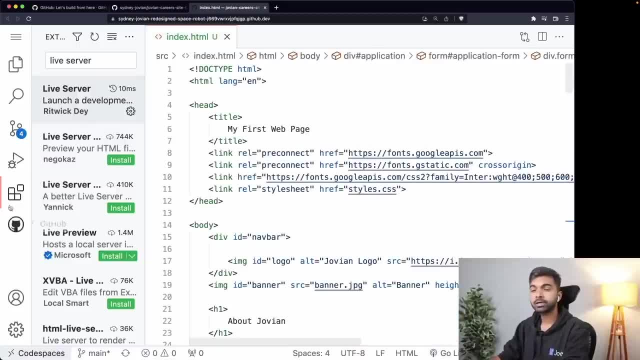 I can close this extension tab and, by the way, the extension menu is here on the left, So in the sidebar it is this fourth or fifth option. Yeah, It's the fifth option in the sidebar, So that's how you come to extensions. 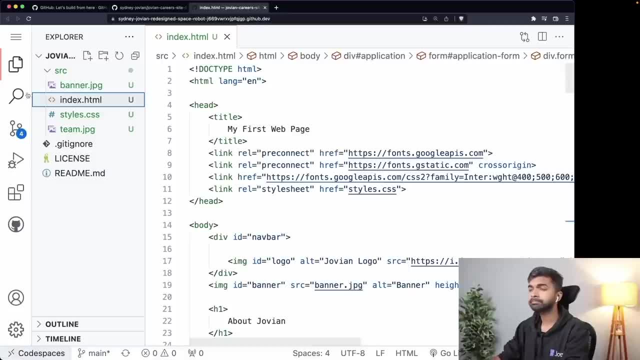 And now, now that I've installed this extension, I can come back here onto my file Explorer And now I can see here that on my index or HTML file- if you see at the bottom here- I have this go live button right at the bottom here. 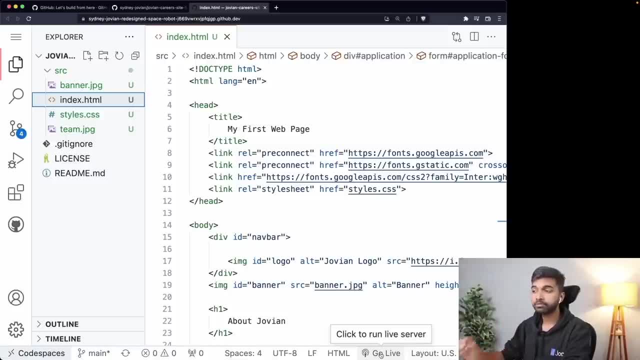 So this is a new button That has been added by the live server. or I can also just right click on index or HTML and I can say open with live server. Both of these are going to do the same thing, So I'm just going to click the go live button. 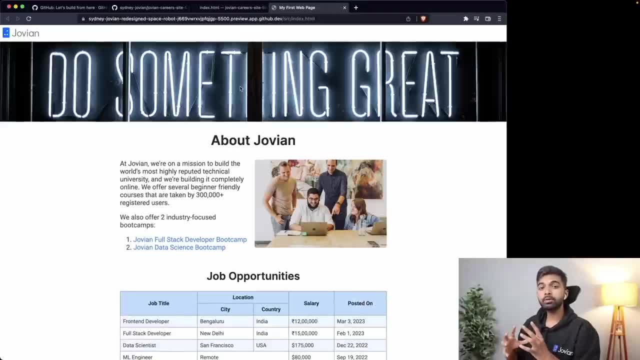 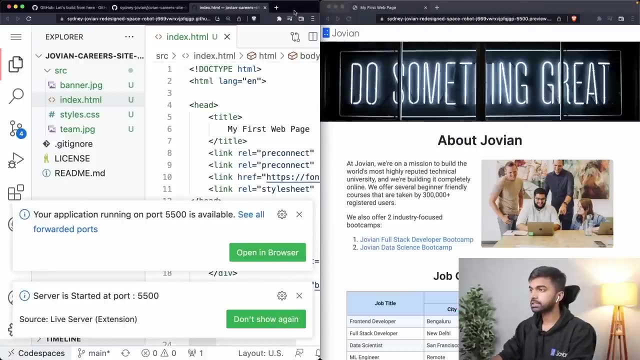 What that does now is it is going to now set up our code space to expose this file to the browser at a separate URL like this: Okay, So now I can. let me put this on the left and let me put this, Yeah. 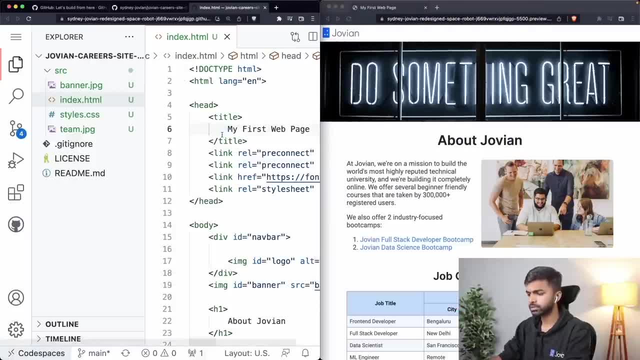 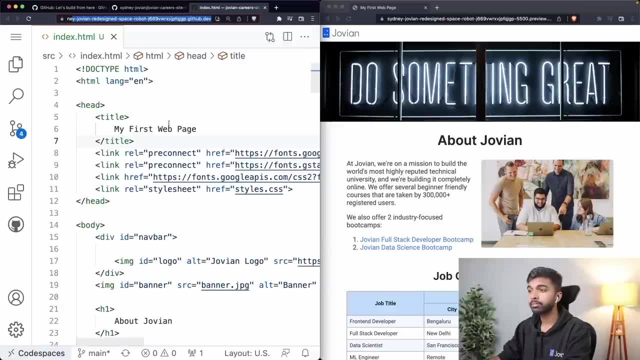 On the left and right And let's close these. Let us also close the sidebar. Now you can see that here I have my code space running on the cloud, So my VS code running in the browser, and I have a live preview of my code running here, open while using the live server. and on the right. 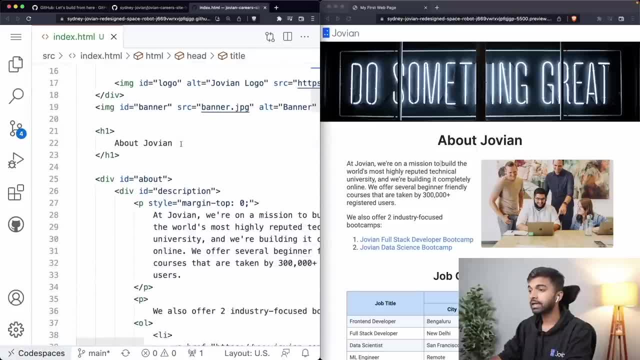 Okay, Now here is one nice thing about the live server. Let's say I want to go back and I want to change here. I want to change about Jovian, to welcome to Jovian, And I just hit save, That goes ahead and that automatically refreshes the page. 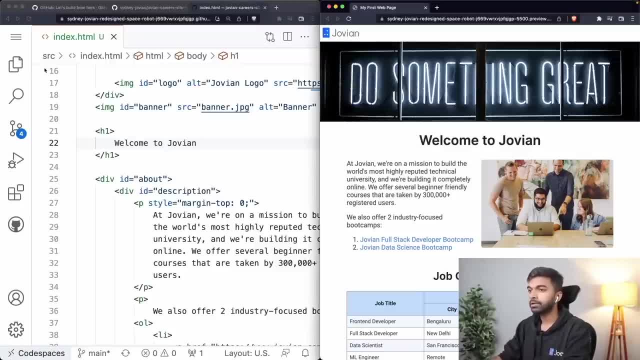 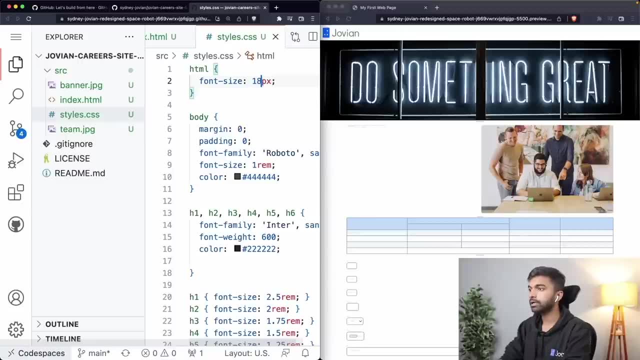 So the live server makes it slightly nicer to develop And I can also go and do this with the style store CSS file. I can say: let's say, change the default font size from 16 pixels to 18 pixels and I can save it. 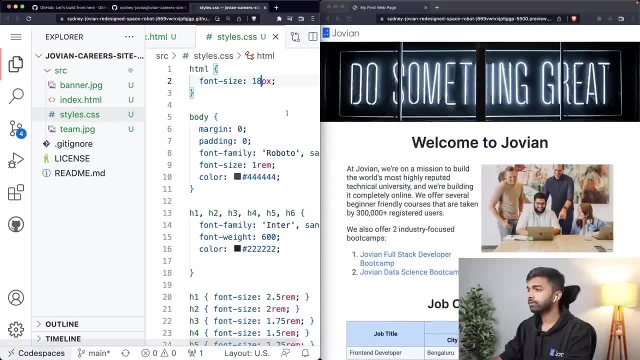 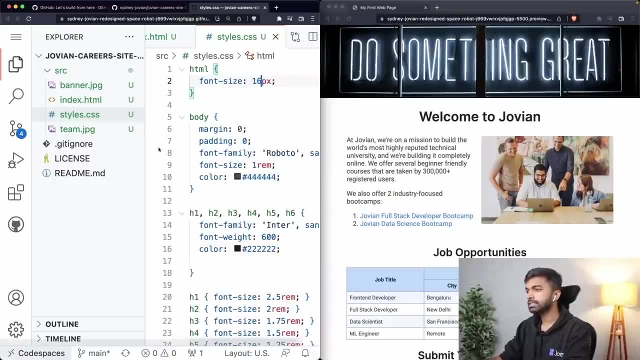 And you can see that now the styles file has been updated and now we have- let's make it- 20 pixels. Maybe now you can see that these things are a lot bigger. Okay, So this is one of the nice things about the live server. 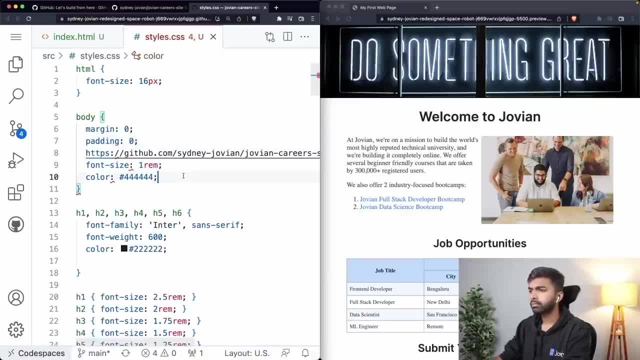 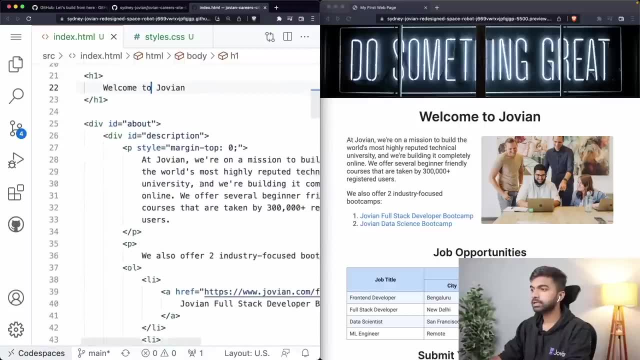 Okay, All right, So, oops, I think I pasted something. Yeah, So this is one of the nice things about the live server. You can go in, you can make some changes here. They can say: maybe I want to get rid of the word highly and I just save, and that changes this automatically. 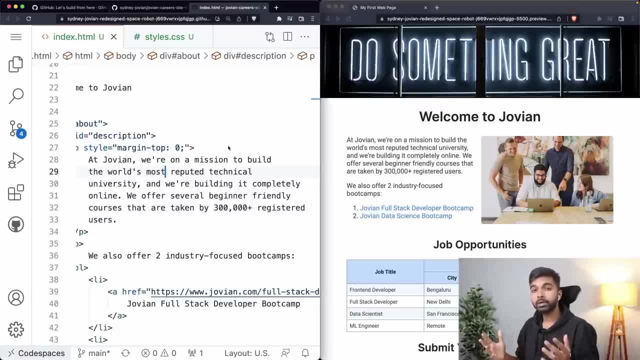 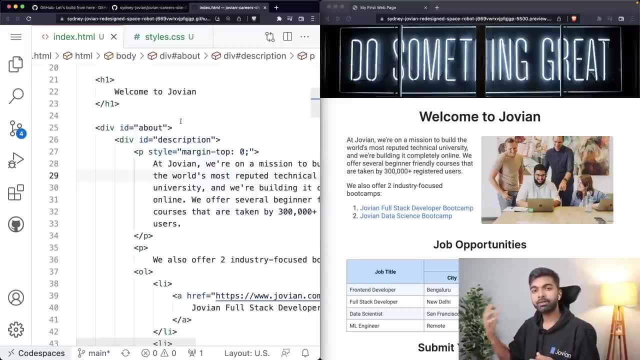 Okay, So that is how you view the code that you are building, that you're writing on, Especially when you're building a simple HTML and CSS page. later on, when we look at web frameworks and things like react et cetera, then we'll touch on. 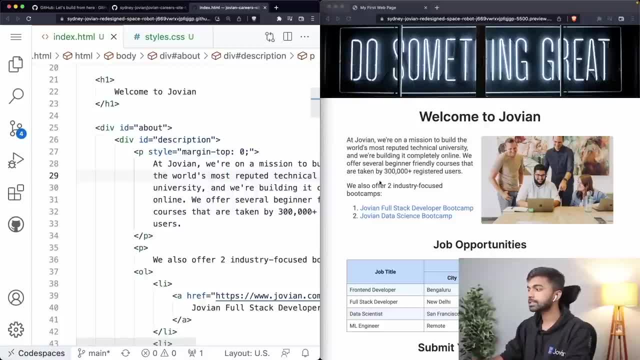 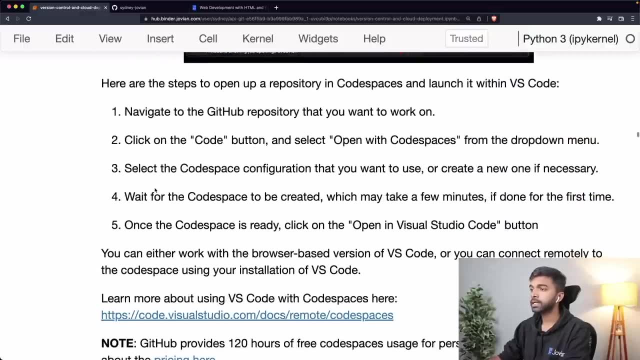 Other ways to look at previews, but on GitHub code spaces. this is how you look at a preview of your code. Okay, So just to quickly recap. to start a code space, you go to the GitHub repository, you click on the code button and you select open with code spaces. 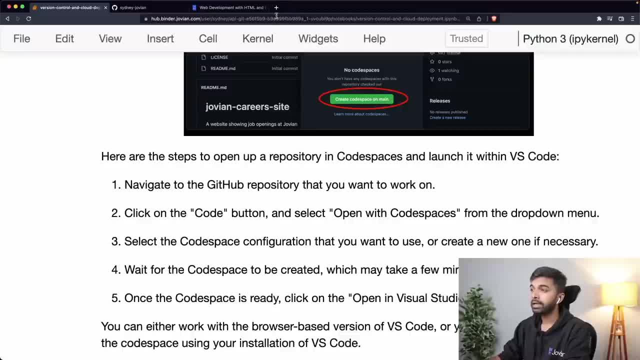 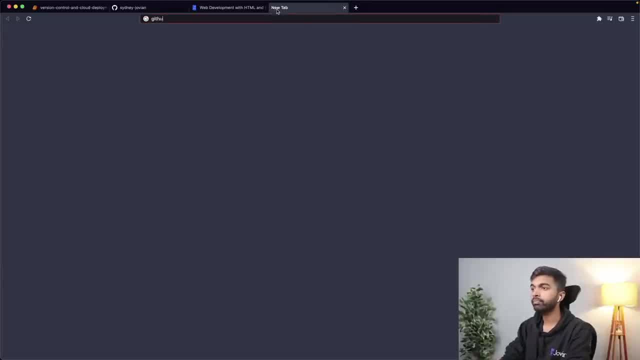 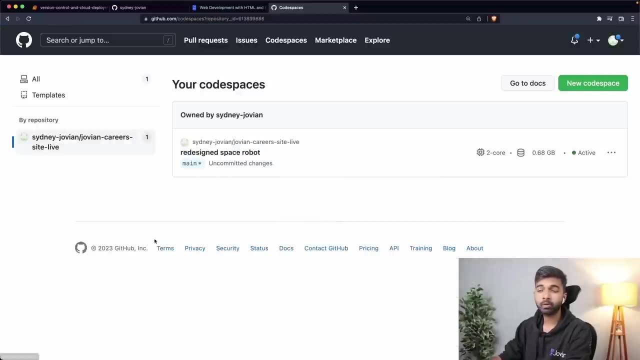 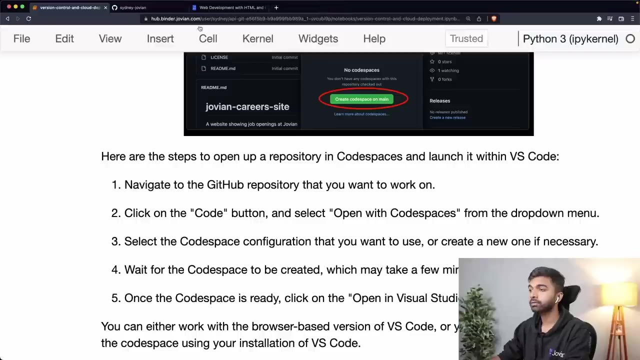 You can create a code space on your main branch if required And if you ever need to. you get two free code spaces. So if you ever need to delete previous code spaces, just go to githubcom slash code spaces And over here you can go into your specific code spaces, repository wise, and you can go ahead and delete them in case you have a new repository that you want to develop using a code space. 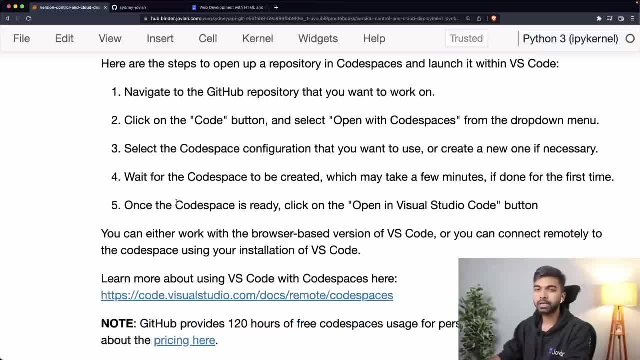 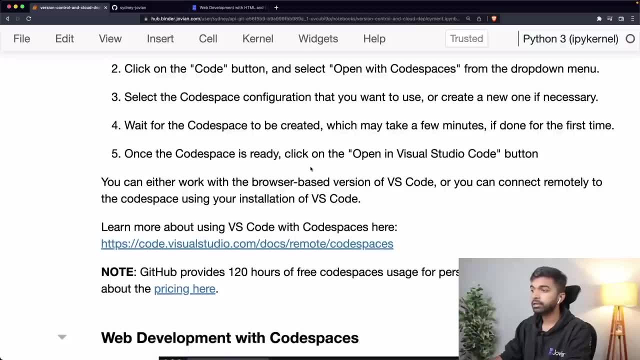 Okay, And then you can select a code space configuration. Typically, the basic configuration should be good enough. Then the code space gets created. It takes 10, 15 seconds and then you can just open up visual studio code in the browser or you can actually also connect your local visual studio code to the code space. 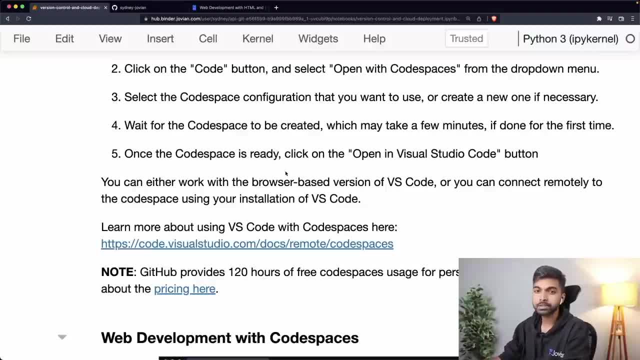 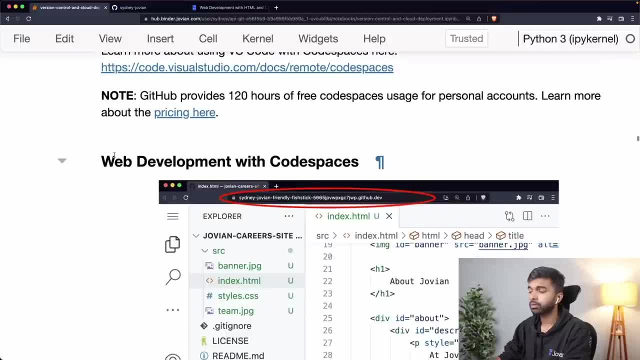 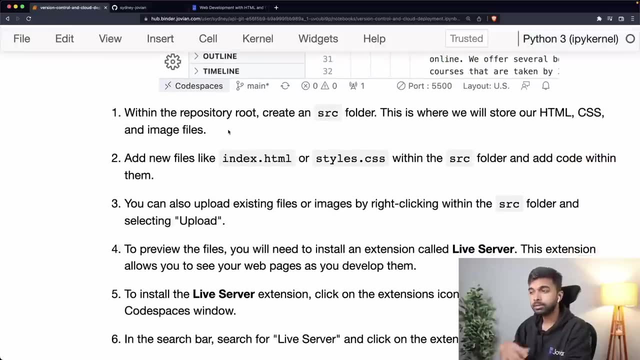 We're not going to go into that today, But, Uh, browser-based development is good enough for most projects, And then you can continue working on your code spaces project. All right Now, in terms of how you do actual development, well, what you do is, you can: uh, one thing that we recommend is that now, anytime you're putting your actual web code, uh, you should create an SRC folder. 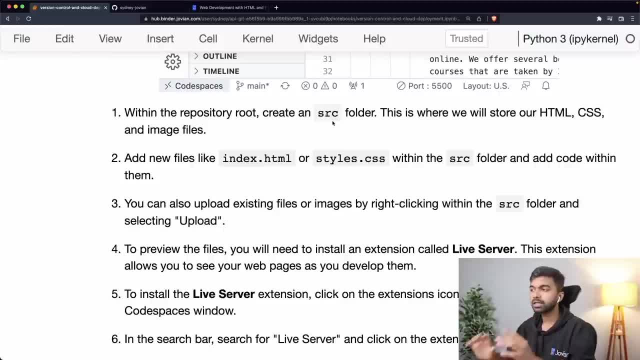 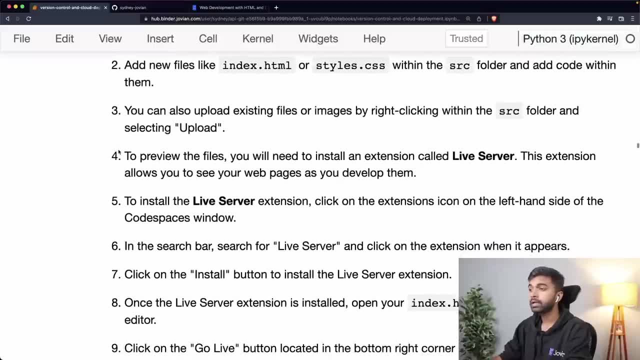 So to separate it out from the read me, get ignored, et cetera, just to keep things clean. And now you can add files like indexhtml stylescss. This is within the SRC folder and you can add code within them. and you can also upload existing files or images by simply right clicking. 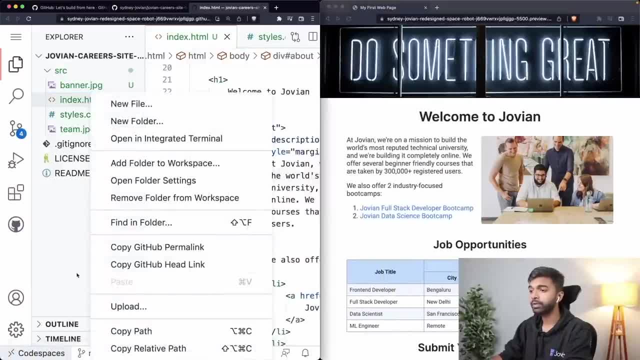 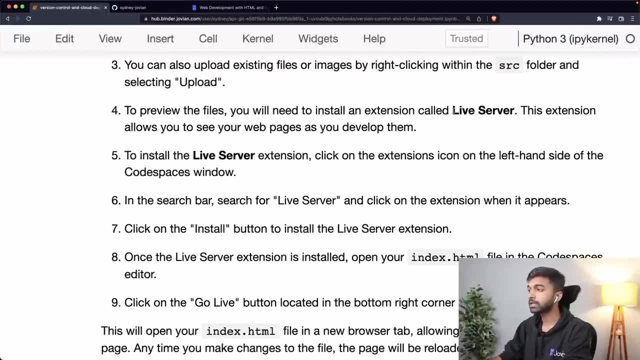 So you can open up the sidebar, right Click anywhere, click upload file and upload a bunch of files. And if you want to preview HTML files within code spaces, you just use the live server extension, and this extension allows you to see your web pages as you develop them. 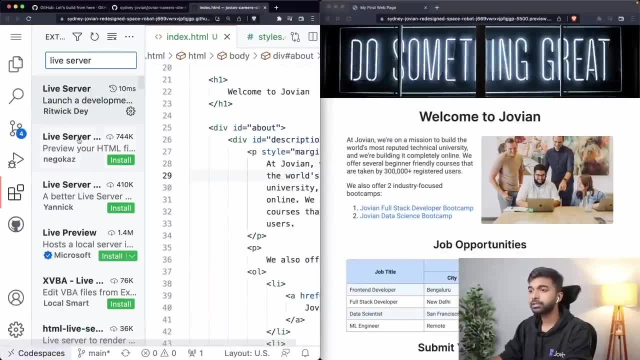 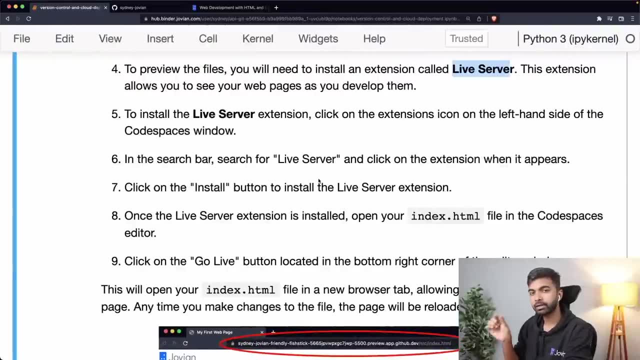 And for that you just go into the extension section here in the sidebar and you search for live server, install it And then you go back and just click go live And you can also shut it down. There's a button right at the bottom to shut things down as well. 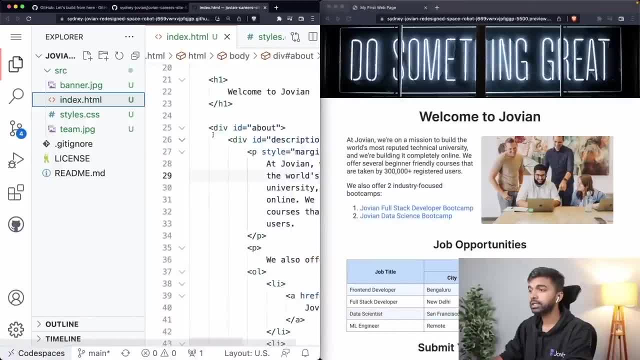 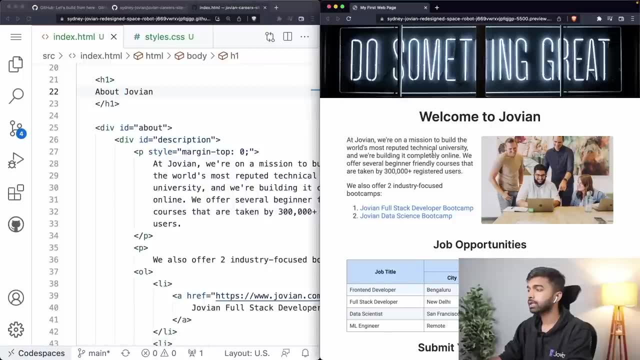 And once you do that, you will be able to see a live preview and you can make changes. For example, if I change welcome to Jovian back to about Jovian, that is going to quickly change over here as well. Now, this is all well and good. 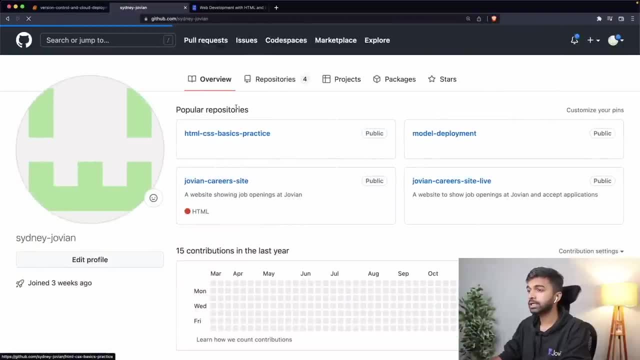 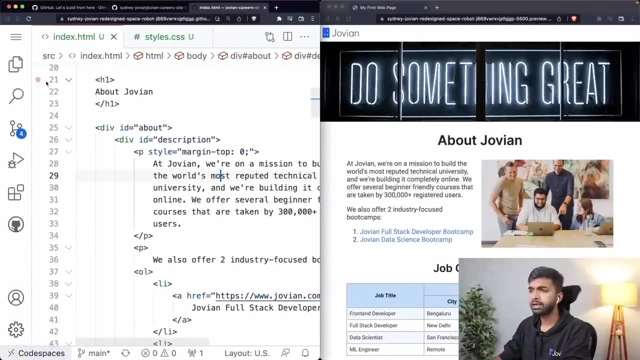 I'm making all these changes, but if I go back to this repository, you will see here that it still does not contain The code, The code that I have actually added. So I've added a bunch of files, but they don't seem to be here in the GitHub repository. 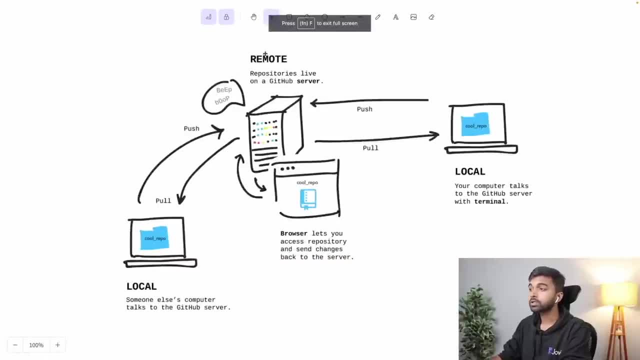 Well, remember this, remember this setup. So we created a repository on GitHub and then we pushed that code or we pulled that code into a code space, which is essentially a remote computer on the cloud, And now you've made some changes into our code space machine using VS code. 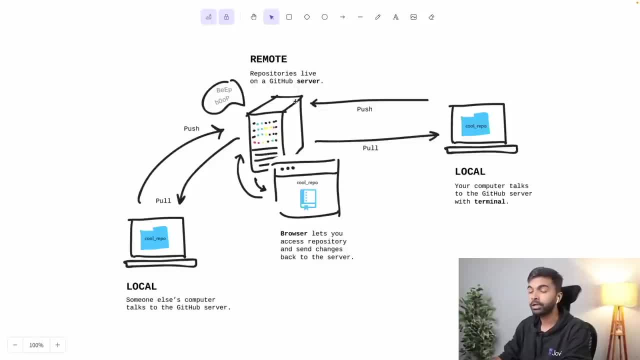 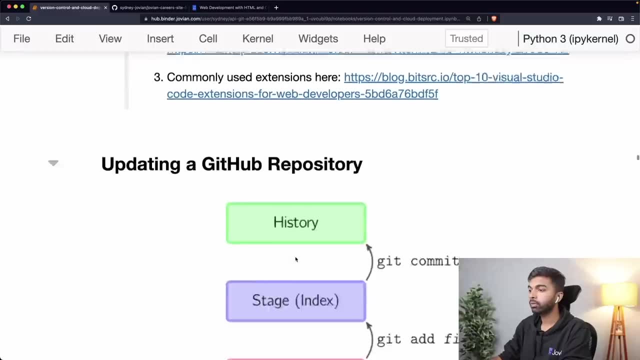 Now we need to push these changes back To GitHub to actually save them back to the remote repository. So that's what we're going to look at next. Okay, So how do we do that? Well, it's a three-step process, and we're going to first stage our changes. 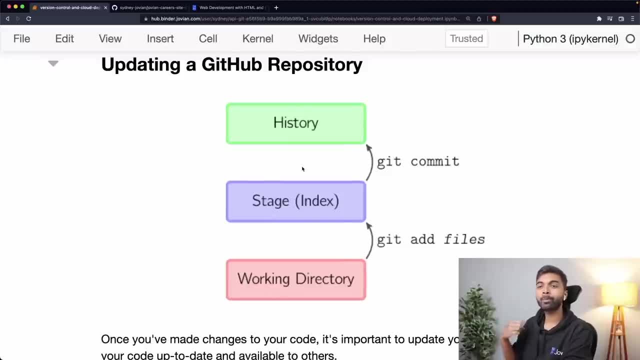 Next, we are going to commit our changes And finally, we are going to push our changes. And this is where some of the GitHub terminology will start kicking in. You might wonder: why do we have three-step process? Why can't I just hit save? 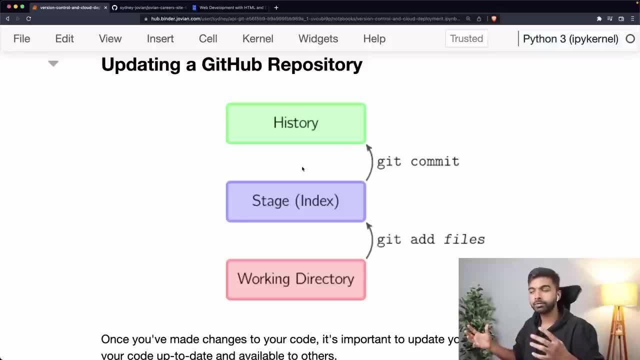 Well, this is just how Git was designed: to handle a bunch of different use Cases, And that is what we are stuck with, unfortunately. but you, once you do it enough, you start to get used to it, And I'll show you some easy ways of doing this without having to type or remember a lot of things. 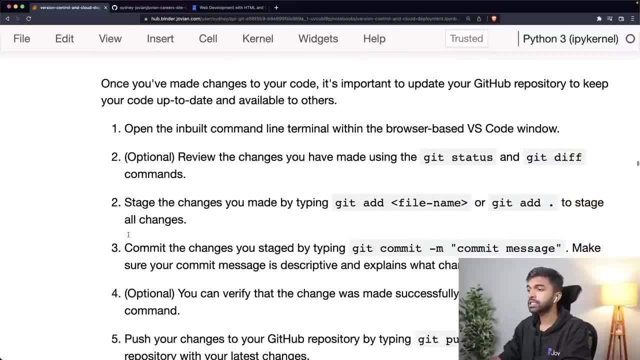 So here is how it works. The first thing we need to do is we need to open up a terminal So get added. score is a command line tool, So you need to actually type out some commands on a terminal or a command line, but we need to open up a terminal to run some of these commands. 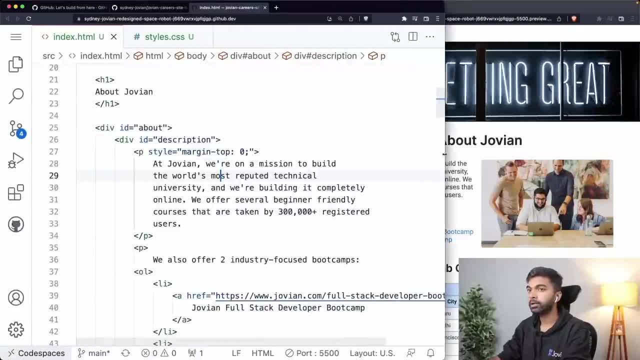 Of course We have our code space somewhere on the cloud here, So we will need. we can't open up a terminal on our computer. We need to open up a terminal on this remote machine which is in the code space. Fortunately, VS code provides an inbuilt terminal. 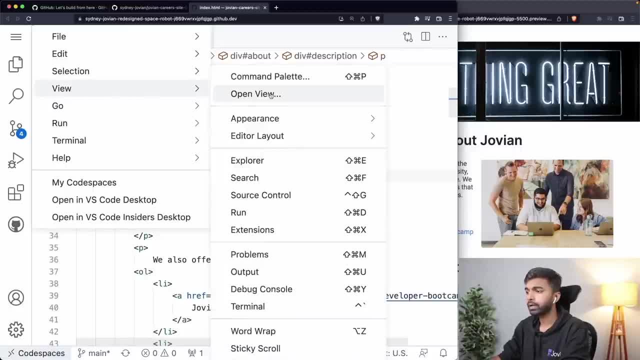 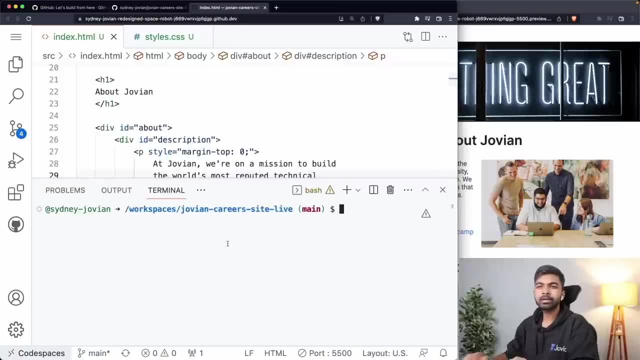 So you can just click on these options here and you can say view, and you can select terminals or view terminal, And now that is going to open up this terminal window. Okay, And what is a terminal or terminal is simply a place where you can issue commands. 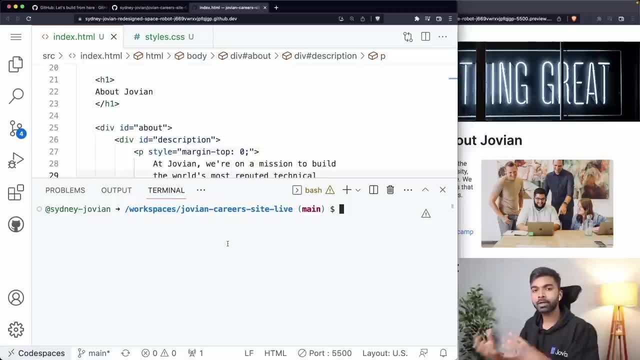 You can write commands And those commands will get executed on the computer. So before we had graphical user interfaces, uh, operating systems were just terminal based, text based platforms where you could issue commands. And even today, most developers use these command line or these terminal commands to run a lot of their code and to interact with the gate, for example. 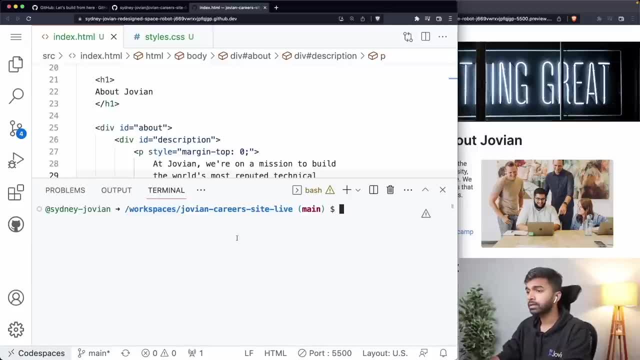 Okay, All right. So now we've opened up this terminal, so it has this. You can see that this Terminal it has a bunch of information already. It tells you who is the current user. So the current user is Sydney Jovian. 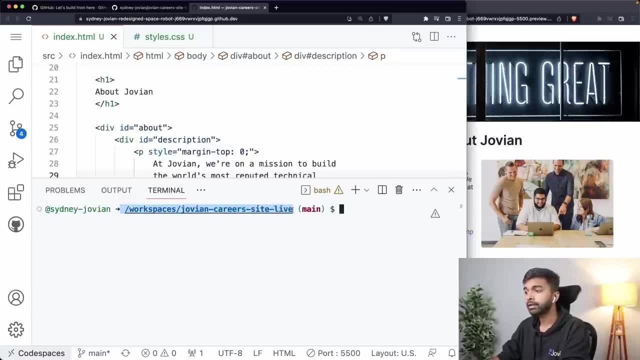 That is the name of our GitHub user. It has the current directory or the current folder on the code space where we are currently at, And it also tells us a branch that we're currently at. So it's an informative prompt. And now, here we can start typing our terminal commands. 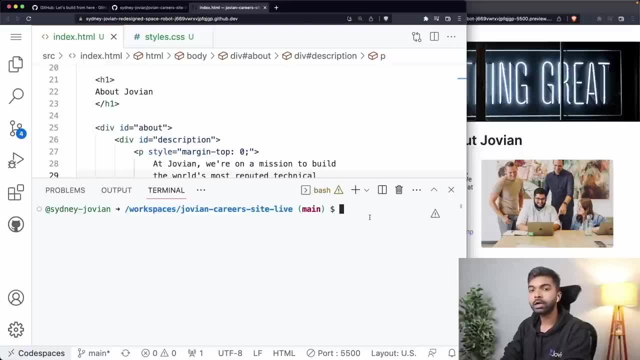 So the first command that we need to do, or we need to type, is called get ad. Okay, So the first thing we need to do is- or actually, even before we do get dad, we can just type Get status to see what status our repository in is in. 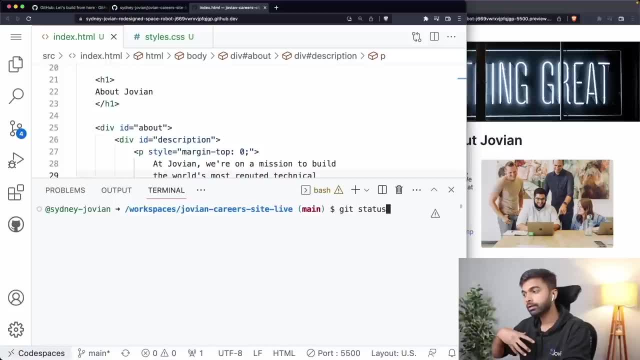 Are there any new changes that we have made since we have Checked out the repository from GitHub. So if I type get status, you can see here that it says that you are on the branch main and then there are a few untracked files. and there are a few untracked files and they are the files in this folder called SRC. 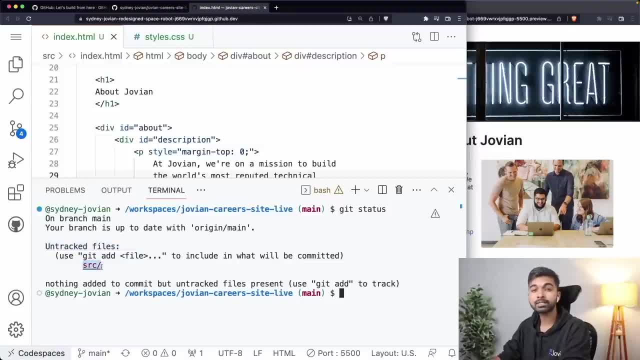 So the entire untracked, the entire SRC folder is untracked. by untracked We we mean that get has no idea about these Files. It has never seen these files before. So the first thing we need to do is we need to stage these files. 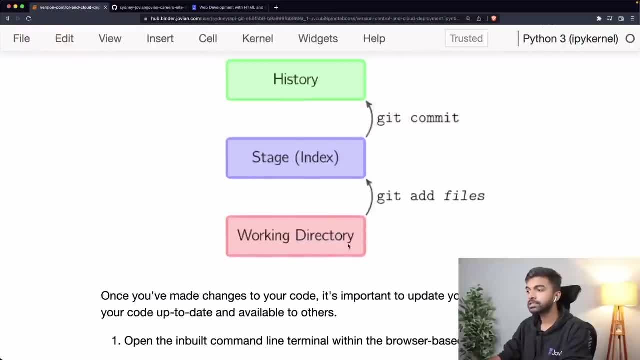 So we take the files from our working directory and we staged them, which means we tell: get that, okay, these are some files that I'm interested in potentially putting to putting back on GitHub. So I'm going to stage them by saying, first of all, I'll just reset it. 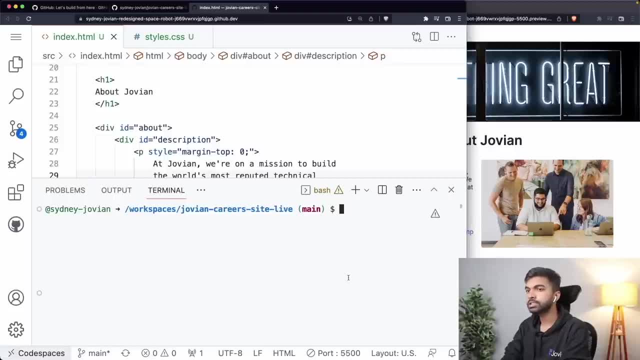 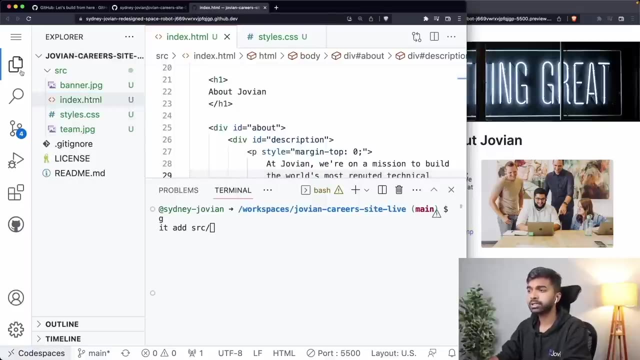 So anytime you want to reset the terminal, just type reset. and I'm going to just stage this by typing: get ad SRC And SRC slash. what are all the files that I want to stage? I want to stage indexhtml, bannerjpg, stylescss and teamjpg. 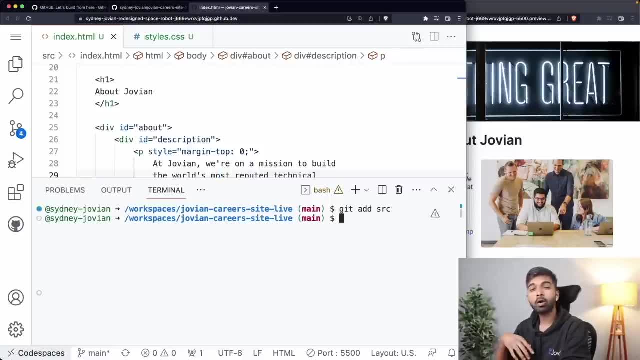 Well, I'm just going to type get ad SRC, and that is going to add all the files present within the SRC folder into the staging area. Okay, So now, if I type get status again, this time you're going to say that it's not saying that there are any untracked files. 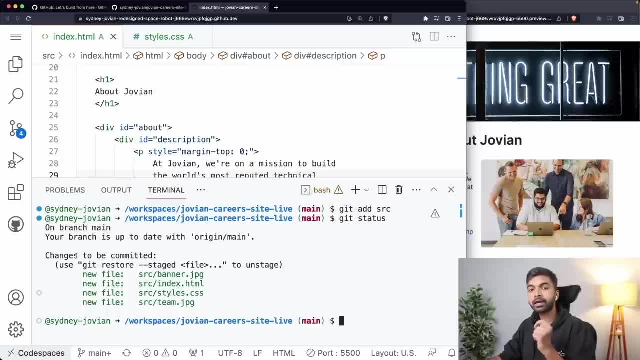 So there are no more untracked files. There are some files which are ready to be Okay. so now in my staging area, which is nothing is yet put into the Git repository. yet we now have a four new files. okay, great. 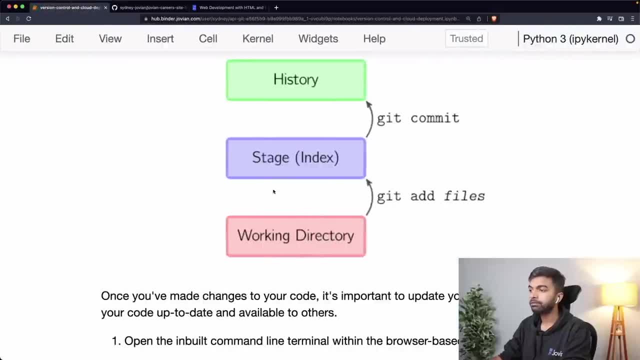 So now that we have staged these files- so from working directory we've staged these files- The next step is to actually record a new version of this entire repository by performing a commit. So here is what we do after adding a Git dot: a Git add. 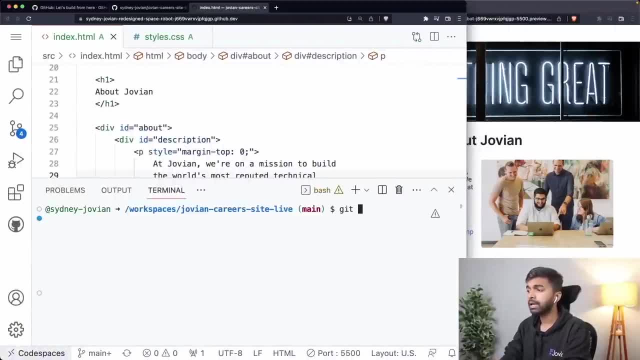 So I've reset things again. Now I type Git commit And then I say minus M and then I provide a message, So adding the HTML and CSS files. Now I have to provide this message within quotations, So we can see here: Git commit. 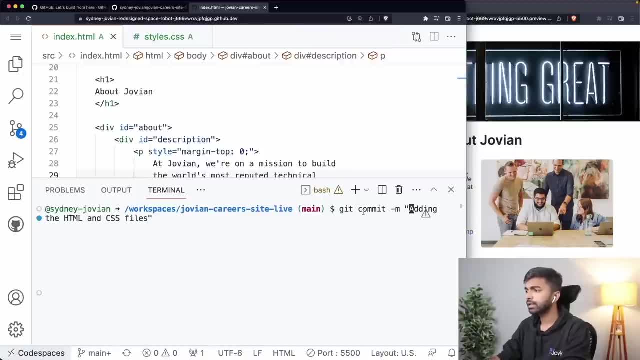 If I have, if I need to zoom in a little bit likely, this is fine. Git: commit minus M, and then I provide a message and the messages within code. So now I'm creating, I'm recording a new version of my code by creating a commit. 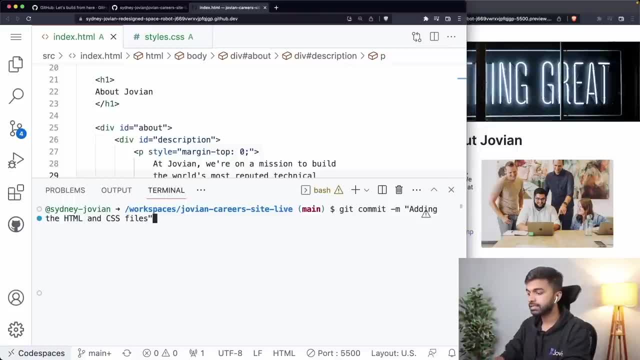 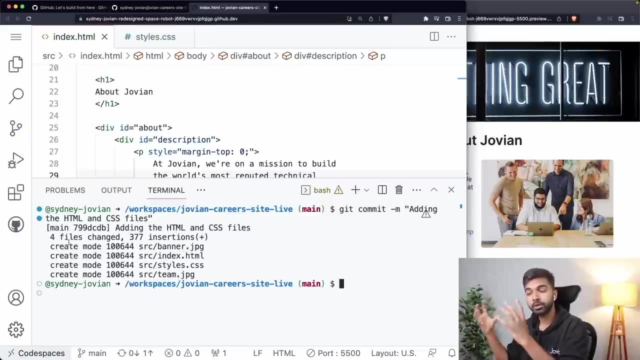 And I'm giving it the message adding HTML and CSS files, and I press enter Okay. And now it says that okay, now it has actually inserted four files into my repository. So now you can see that now we have the create mode. 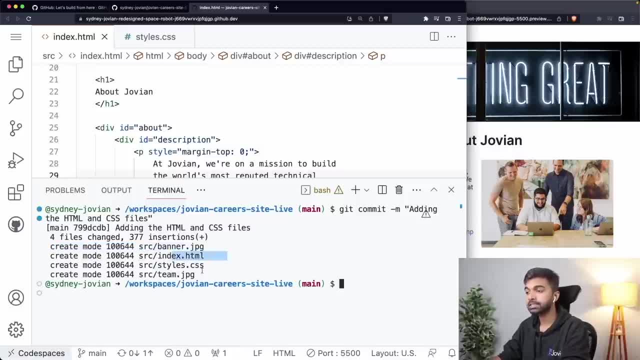 Now we have created a file called SRC banner dot JPG, index styles and team dot JPG. Where are these files created? They were already present on our code space. Well, they have been now created and saved within our repository. formally saved, Okay. 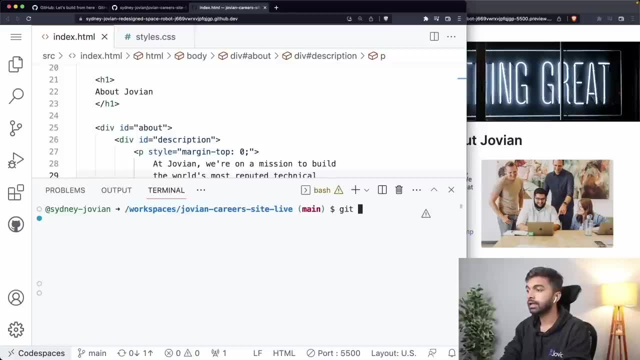 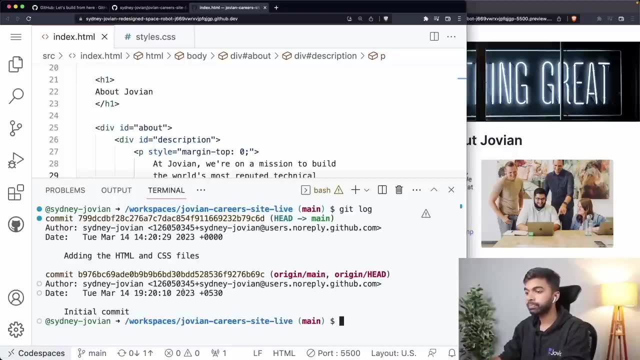 And now, if I reset once again And I say Git log, now Git log is used to view a history of all the commits And now you can see that there are two commits, or two times that I've recorded a version. a commit is simply a version of the code. 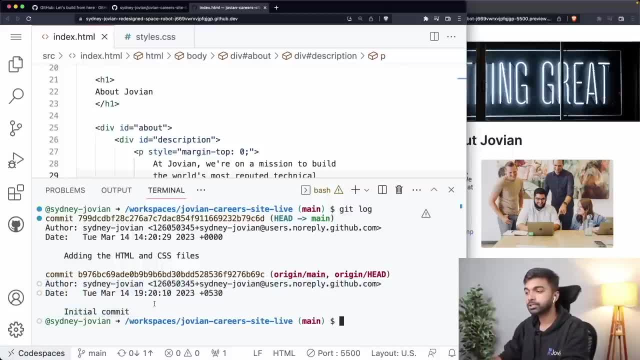 So there was this initial commit that was done at such and such time by such and such author. The initial commit was done and then I have done a second commit, And in the second commit I have added this: HTML and CSS files. So that is also something you can see. 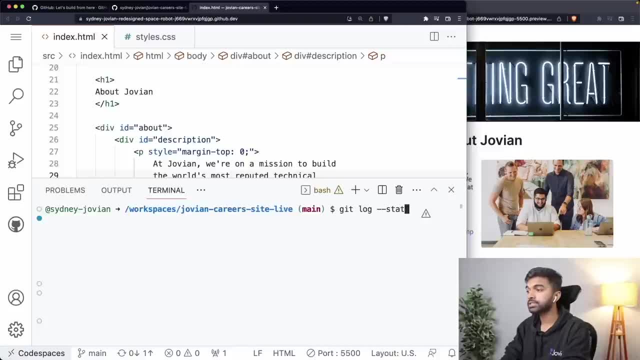 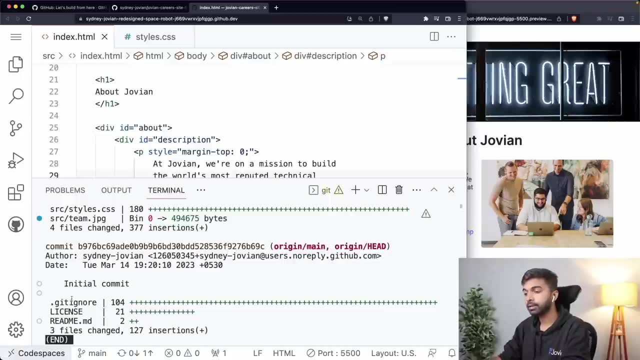 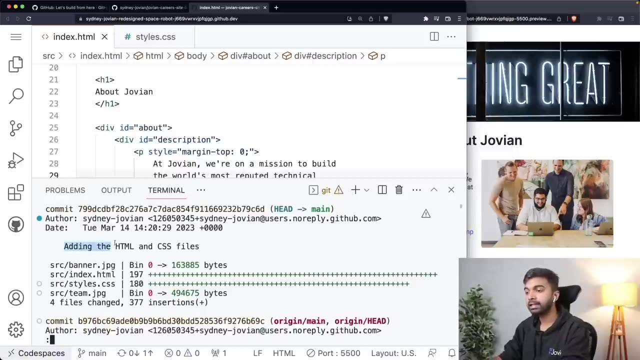 Okay, You can in fact do Git log minus, minus stat, and that is going to tell you what is the change in each commit. So here you can see that in the initial commit we added a Git ignore, license and readmemd file. So I'm just using the arrow key to go up and down and in the new commit adding: 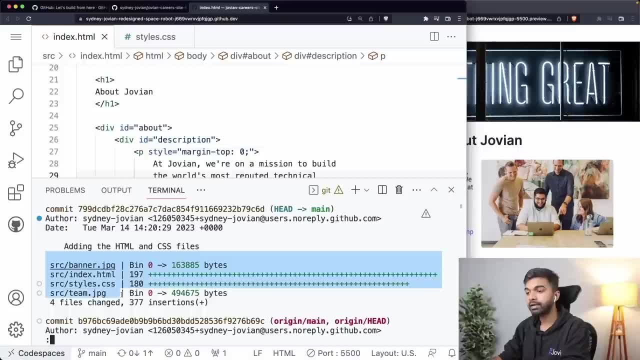 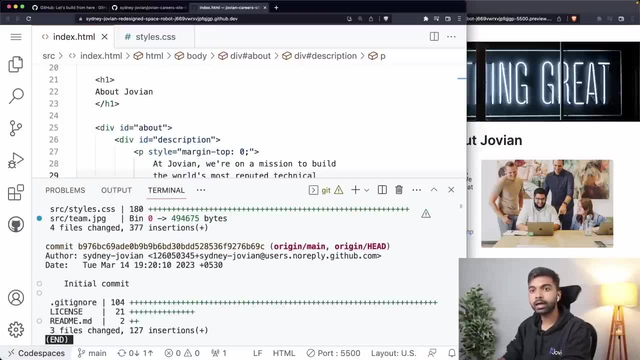 the HTML and CSS files I have SRC banner index styles and these are the number of lines in each of these. Okay Now, often when you run some Git commands, you will have to do this scrolling using your cursor, Up and down cursor. 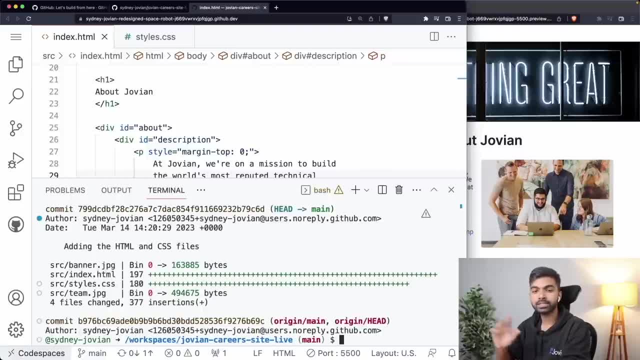 So use a quick trick to exit this: just type Q to exit this, Okay. Anytime you're stuck in some Git command output, just press Q and you should be able to exit All right. So let me reset that again and let us check Git status. 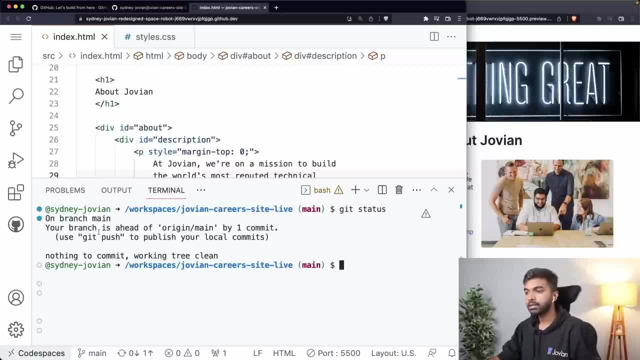 So now it says we are okay, We are on the branch main and there is nothing to commit. Our working tree is clean, which means we have no untracked files. We have no tracked files with Okay, With changes to be committed. 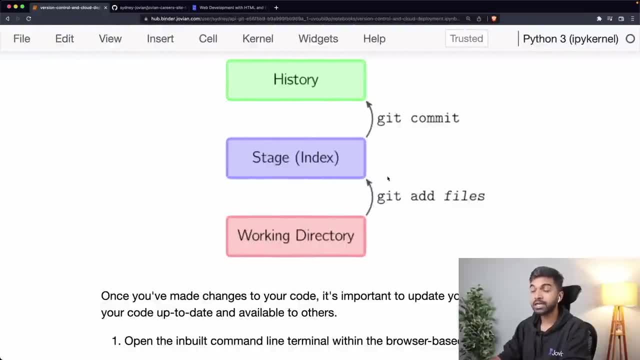 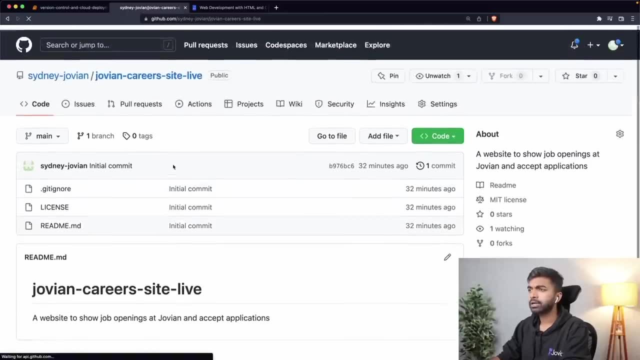 So that's fine. So we have taken our working directory changes. We have first staged them And then, after staging, we have committed these files. Let's see if these have shown up on GitHub yet. No, these do not seem to have shown up on GitHub yet. 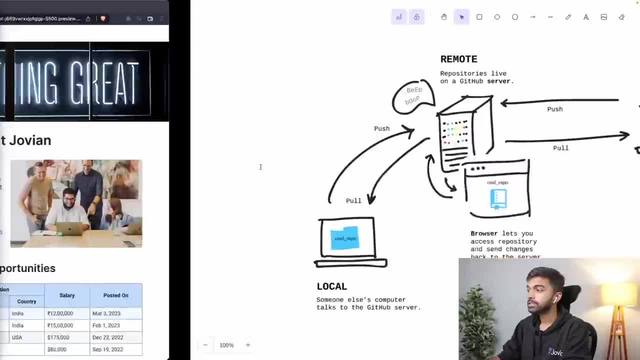 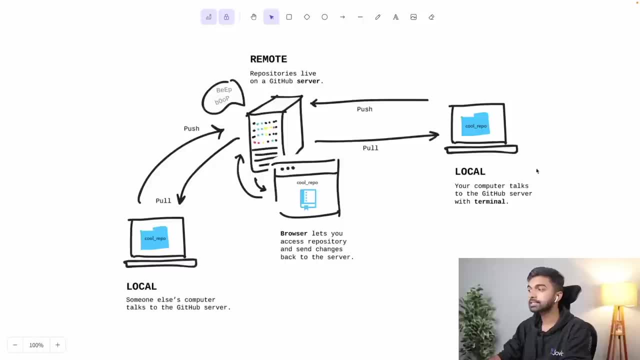 We still have a Git ignore. We still have a license and a readmemd. So, once again, coming back to this, what we are doing here is: so far, we're still just recording new versions of our code on this code space machine. we need to push. 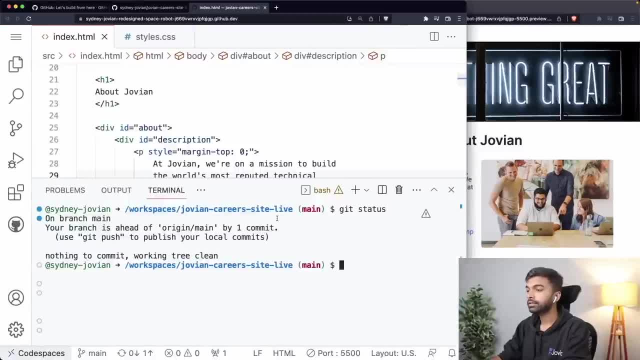 these changes back to GitHub. That is where the Git push command comes into picture. And you can see here there is actually a hint here saying that your branch, So our main branch, the main branch on our code space, is one commit ahead of origin. 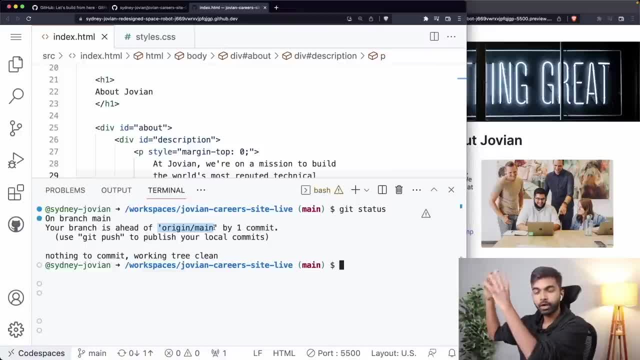 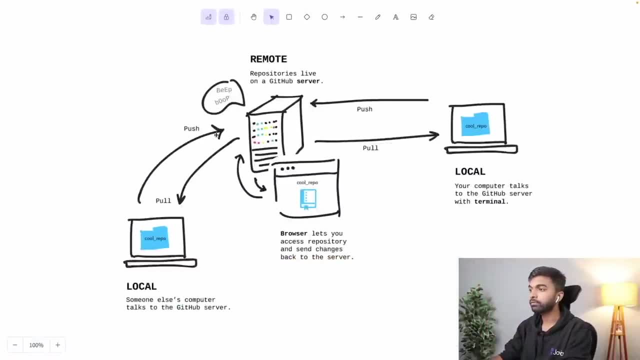 Main origin typically refers to the remote server, the whatever repository remote server from where you've actually pulled this code. So we are ahead of our origin, or we are ahead of the remote server by one commit, So we need to push Our commits. but here's how we push it. 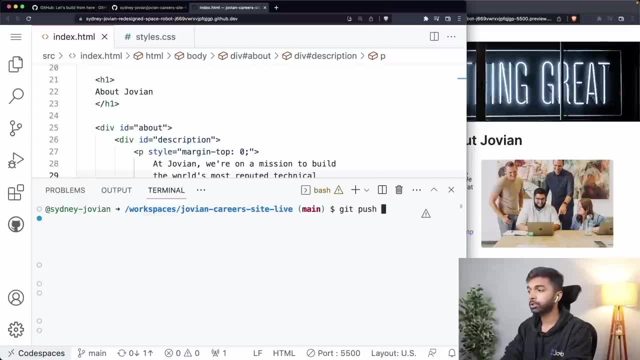 Let me reset that again. Let's just type Git, push and then we provide origin. So we want to push to origin, which is sort of the remote server, and we want to push the main branch. So gate push, origin mean and I press enter. 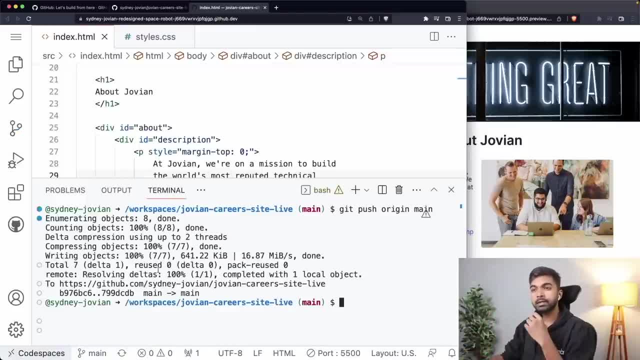 And now you can see that we are packaging up all of these new, new changes that have been recorded in the new commit and we are pushing this to the cloud server. Okay, So now what happens is we have made some comments here. We've pushed them back to GitHub. 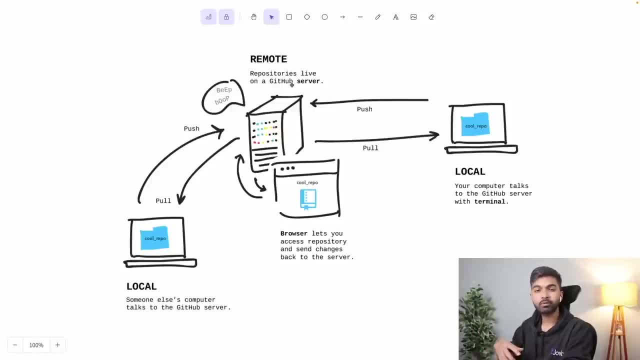 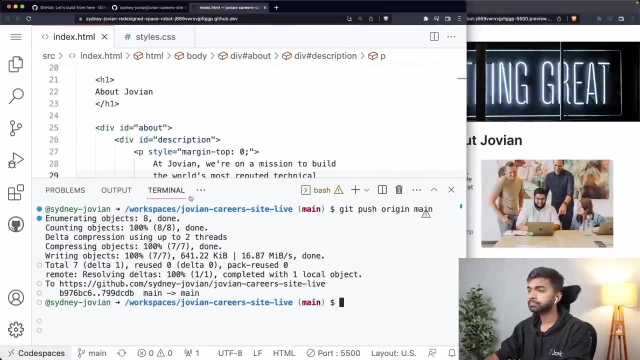 And now, the next time we run a code space or somebody else runs a code space on the same repository- a collaborator- maybe they are going to pull the latest changes, All right, So that is how you actually push your changes back to GitHub. 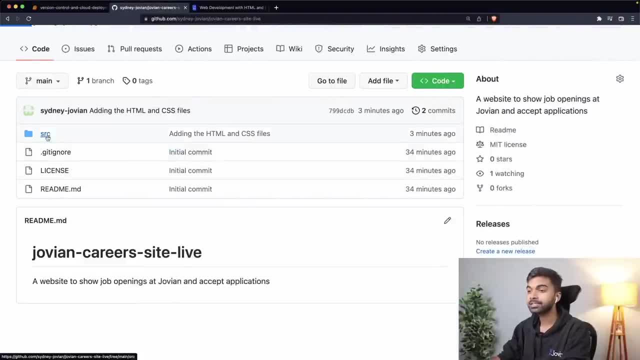 So once again, I reload the page and now you can see. now, finally, we have this SRC folder over here and in this SRC folder we have this indexhtml file. Okay, Okay, Okay, Okay, Okay, Okay, Okay. 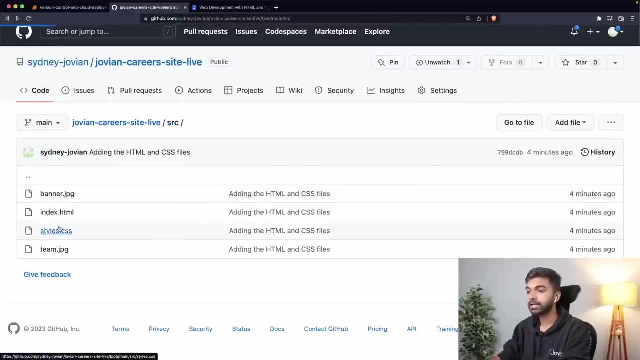 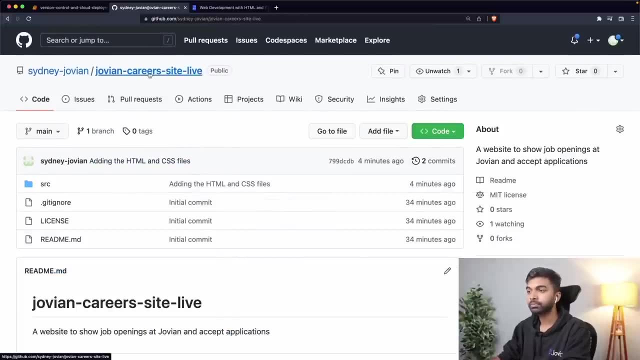 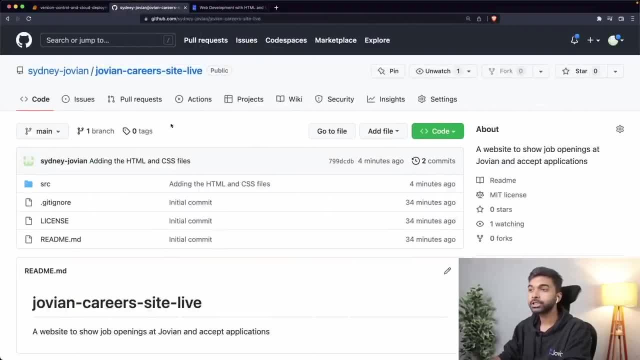 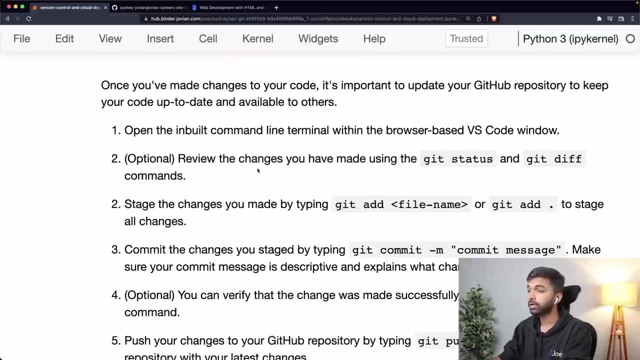 Sorry about that. So that is one way in which you push your changes back to GitHub. So just to recap, you open up the inbuilt command line terminal using the browser-based VS Code window. Then you review the changes that you've made using git status and git diff commands. 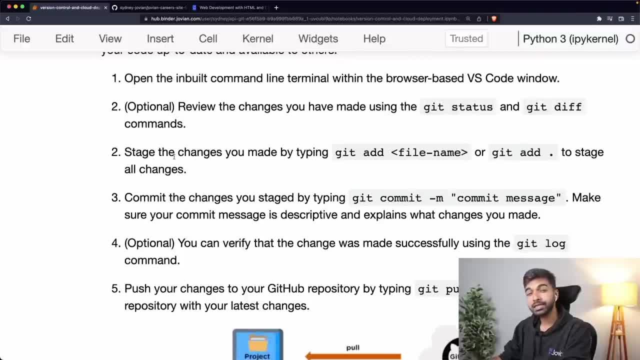 Okay, I'll talk about git diff in a second. then you can stage the changes that you have made by typing git add a specific file name. or you can just type git add dot And that is going to add all the files that have been modified or added. 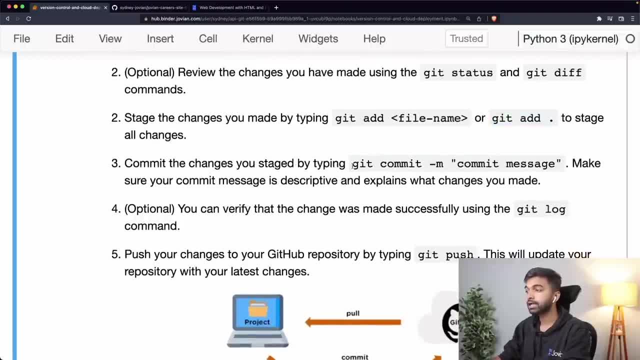 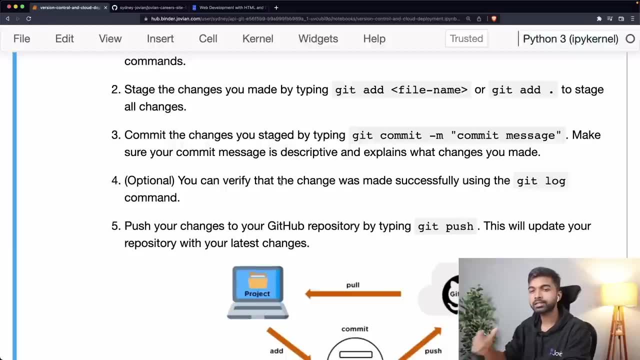 Then you can commit your changes, the changes that you staged, by typing git commit minus m, followed by a commit message inside quotations. Commit messages are very important because they give you a short description of the change you're making And, finally, you can verify that the change was made using git log. 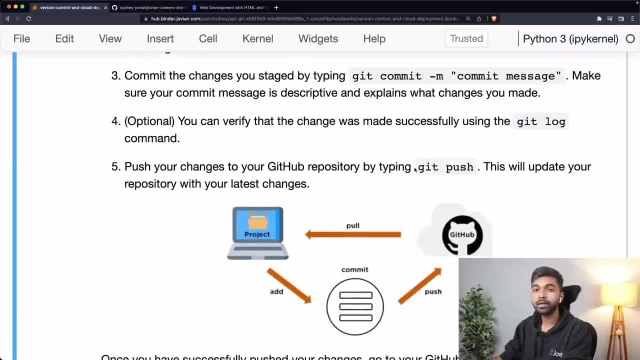 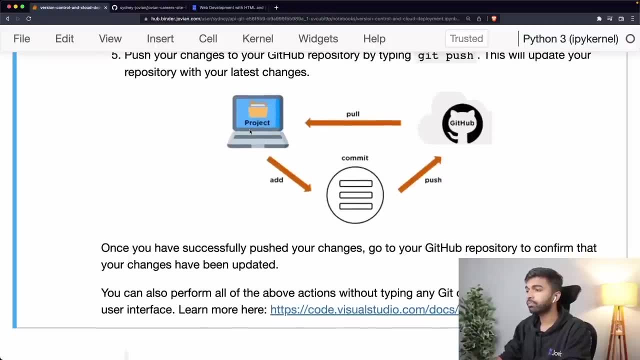 Okay, So you can push your changes to GitHub by simply typing git push, origin, main or, in the case of the main branch, you can just type git push. But this is typically the workflow you have: You add some files, you commit them and then you push them. 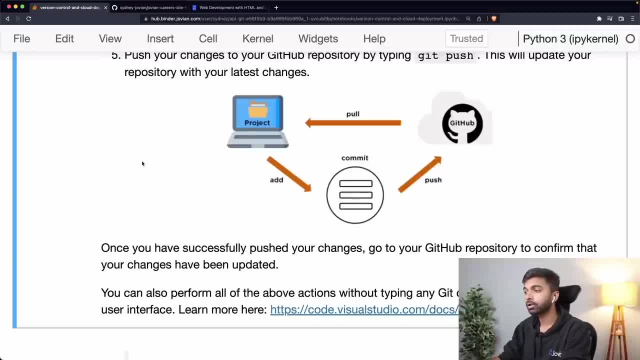 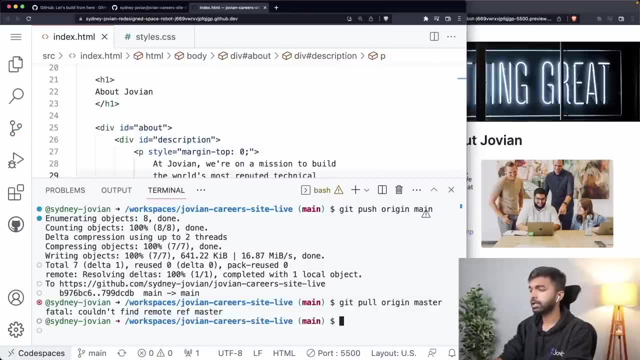 And if there are new changes that are made on GitHub, you pull them back onto your computer. Okay, So if I run git pull origin master, for example, you will see that. or, sorry, git pull origin main. So if I run git pull origin main, for example, 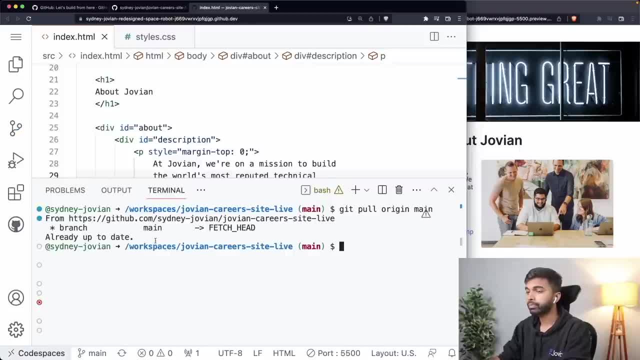 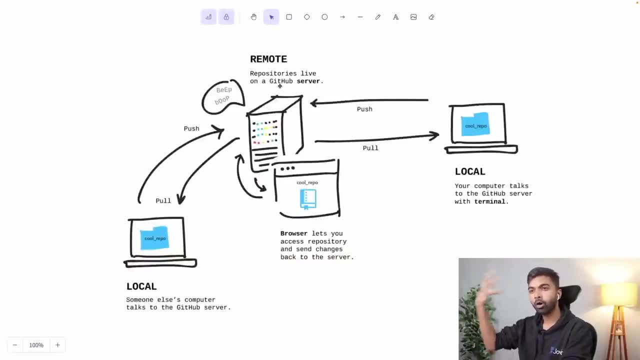 You will see that I'm already all up to date. Now, what is origin? Origin simply refers to that remote server from where you've pulled the repository originally. So it is the origin of your code. it is the original place from where you've pulled your. 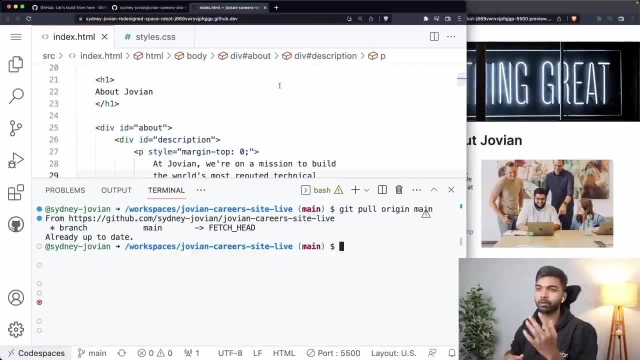 code. Okay. And again, this is where git gets confusing: of origin, remote, this and that, But that's what origin means. Okay. Now, one other thing I want to tell you is, let's say, we make a change here. 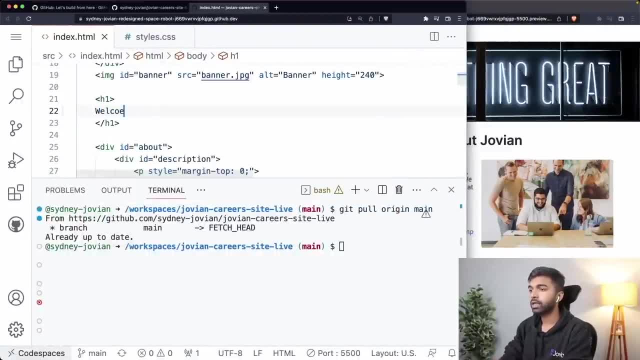 So we say about instead of about German. Let me change this. Let's go back to welcome to Jovian. So the live server should also reload to show welcome to Jovian. And now just to quickly recap the flow: I can check git status and you can see here: 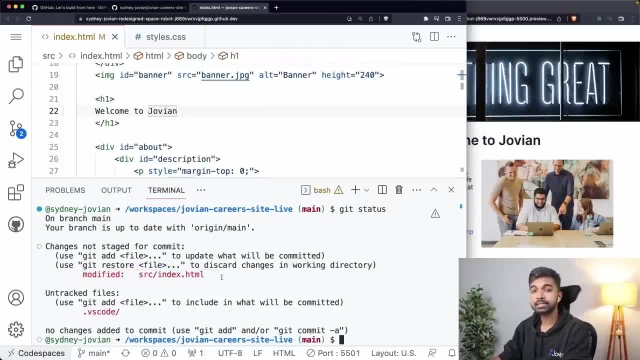 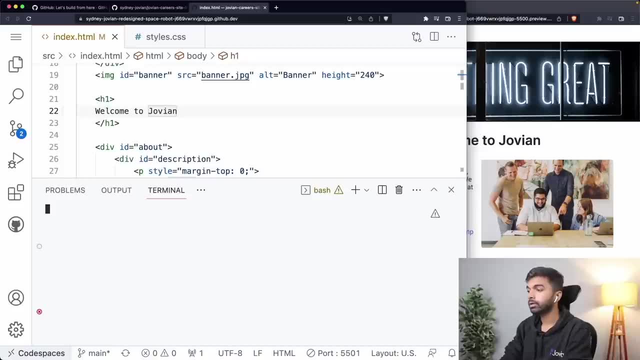 that now we have modified the, now we have modified the file src, slash index dot HTML. Okay, Now it is telling me that something has been modified. Now, whenever a file is modified, you can actually see what changes have been made by typing git diff. 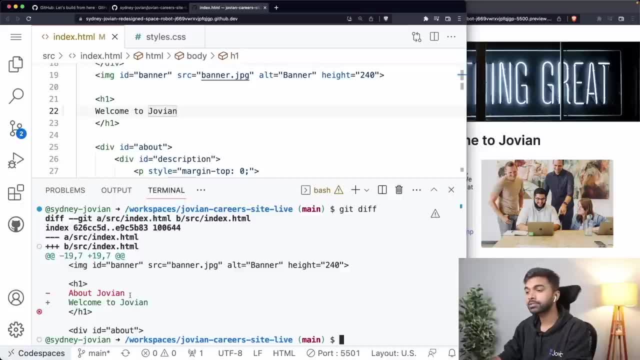 When you type git diff, GitHub is going to show you: In red it is going to show you which files have been removed, which lines have been removed, And in green it is going to show you which lines have been added and everything else. 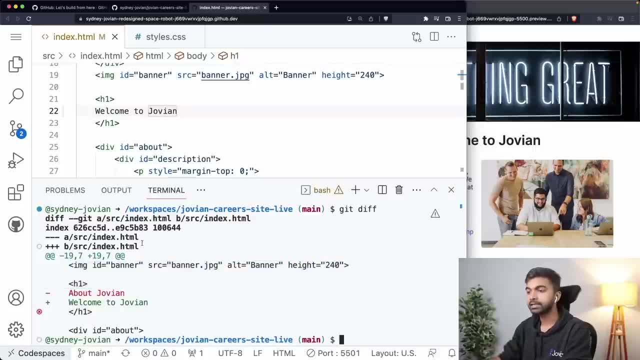 in black is simply the code around that line. So it is telling us that in index dot HTML we have removed one line and we have added one line. Okay, And that is how GitHub tracks, or git tracks, changes. It tracks deletions from a file and it tracks additions from a file. 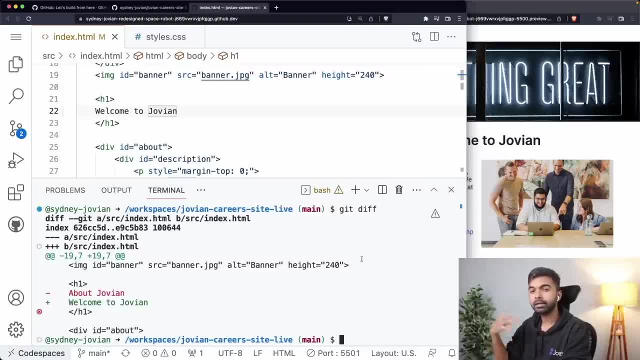 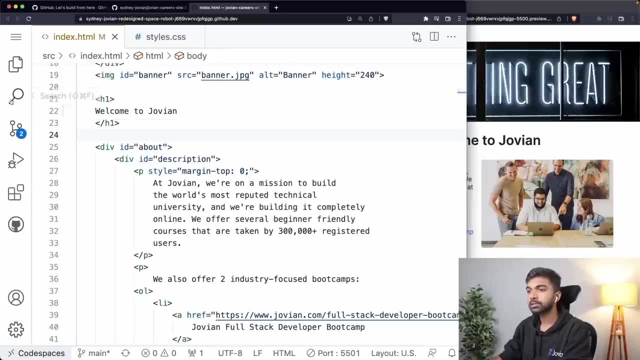 Okay, And once again we can now do git, add dot, We can then commit, We can then push. but there's another way to do it, directly within VS code. So you can click on this third button here, called source control, in the sidebar. 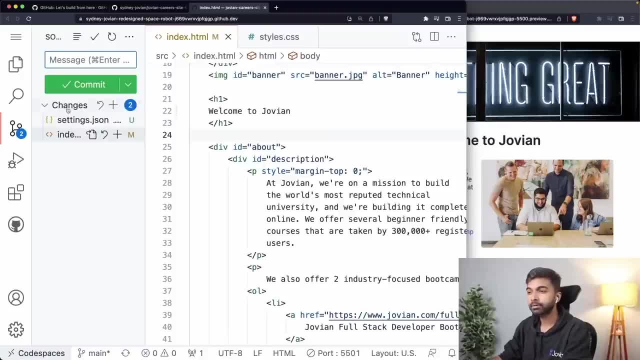 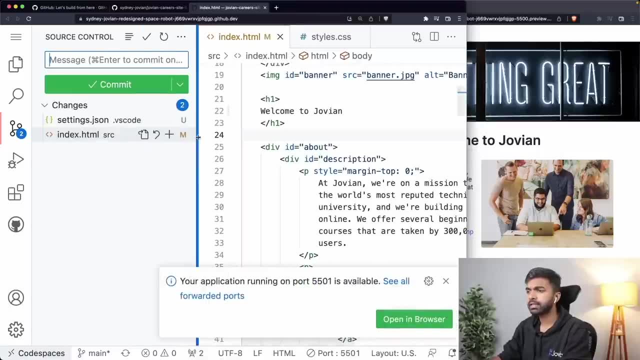 And what this tells you is. this shows you under this changes section. it shows you all the untracked or modified files. So it seems like there is this index dot HTML file that seems to have been modified, And there's also the settings dot JSON file. 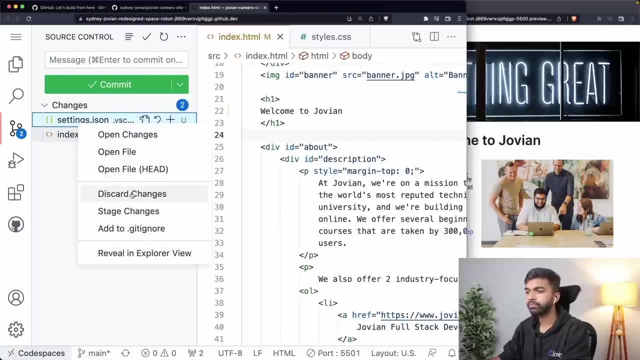 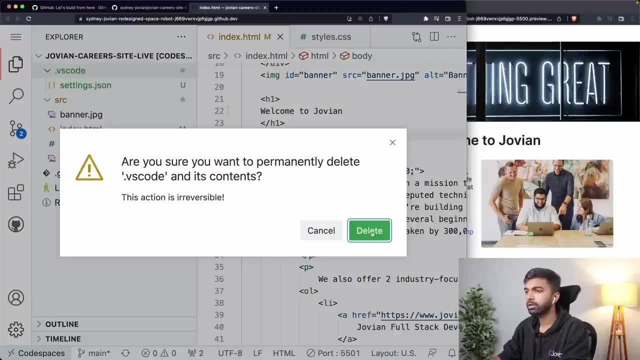 Well, maybe I don't need this file, so I'll just delete this file for now. Let me just come back here and let me just delete this entire folder. Maybe it got added somehow. I don't need it right now, but anyway, coming back here, 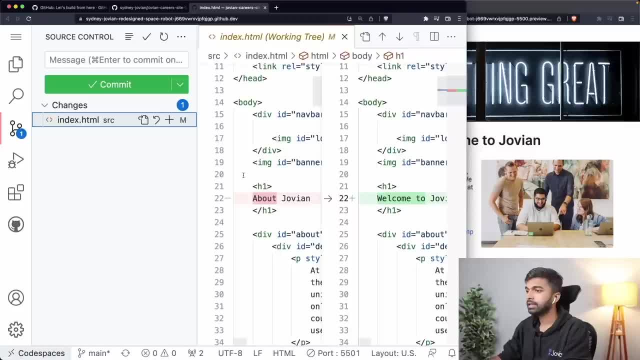 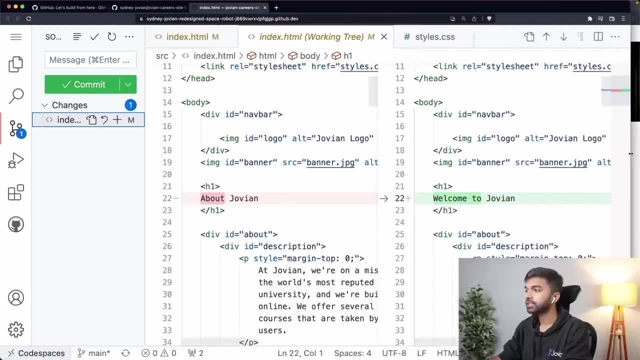 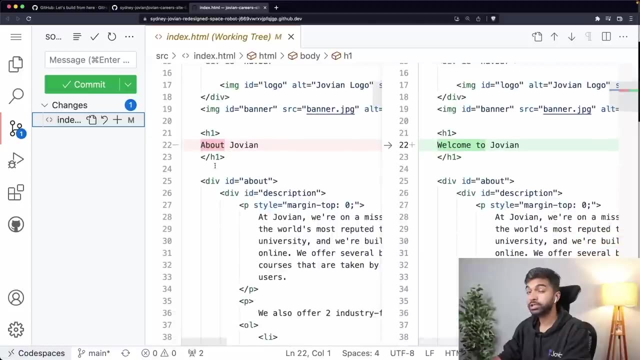 So now I have this index dot HTML file and in this index dot HTML file, if I click on it from the git sidebar, I will be able to see the changes that have been made. So you can see that in index dot HTML it is showing me a comparison between the original. 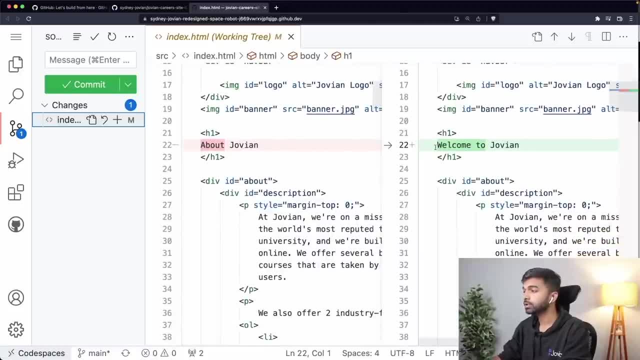 version which contains about Jovian. Okay, To the new version which contains welcome to Jovian. So we have removed about and we have added the welcome to, or you could also think of it, as we've removed this entire line and added this entire line. 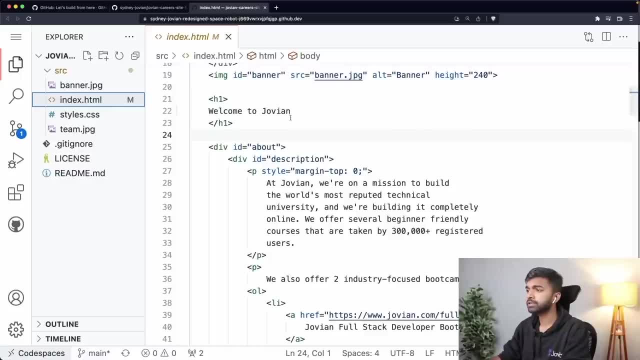 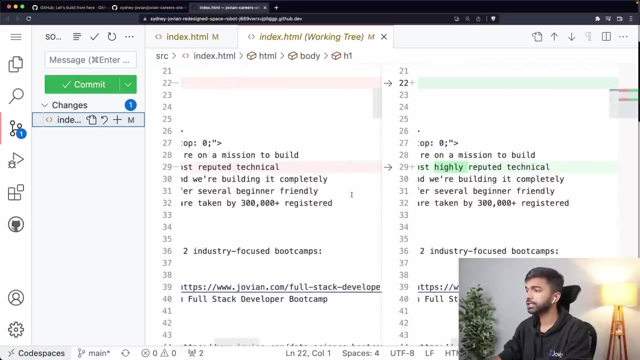 Okay, If we made some more changes, for example in index dot HTML, let's say: let's also remove, Let's also add the word most highly reputed, and let us come back here and let us check. You can now see that, apart from this one change, we also have the second change over here. 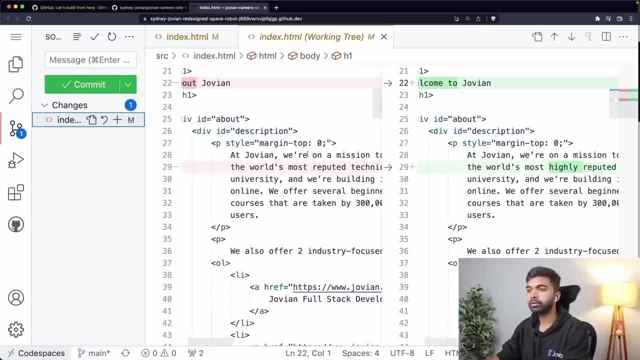 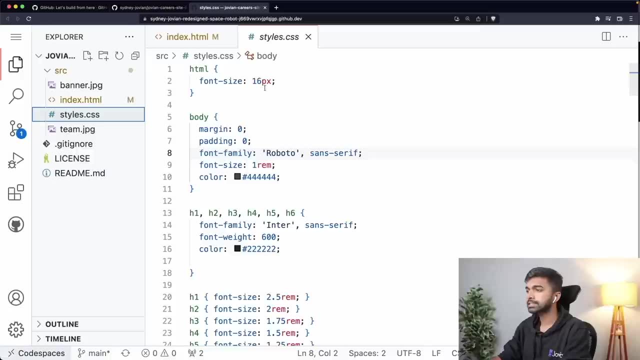 So you don't actually need to run. If you want to do a git diff command, you can simply come in into the into the git sidebar, and you can check the changes. Let's maybe go back and also make a change into styles: dot CSS. 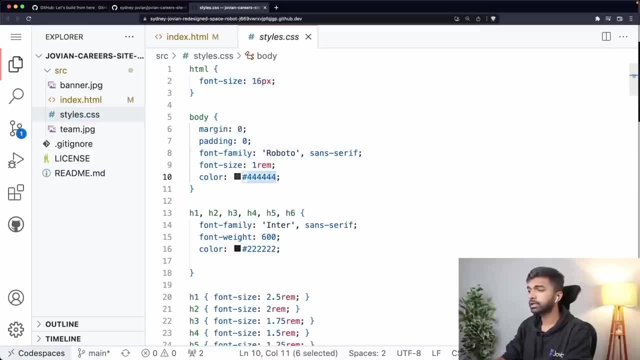 Let me change the body font color. instead of four four four, Let me change it to four zero, four, zero, four, zero. slight change, And once again I can go here into the git sidebar and I can see that there is a change. 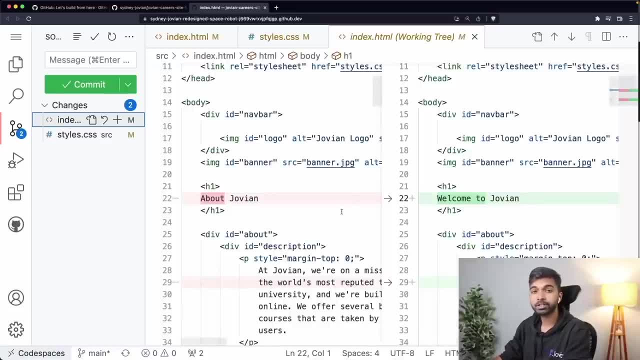 made in styles- dot. CSS. And there is a change made in index- dot HTML. Okay, Now I can go ahead and stage these changes one by one, So I can review the changes in each of the files by looking at the diff or the differences. 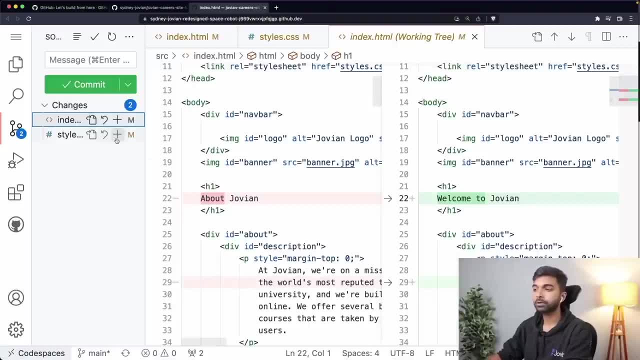 And then I can stage these. I can click plus here and I can click plus here. So remember the flow. we first have to add the files, to stage them, So I can click plus and styles has been staged, or I can unstage it like that. but let me 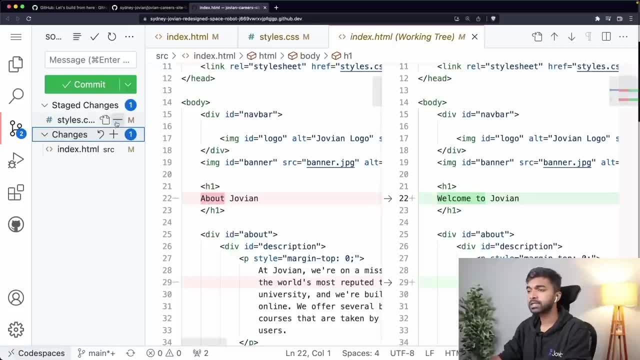 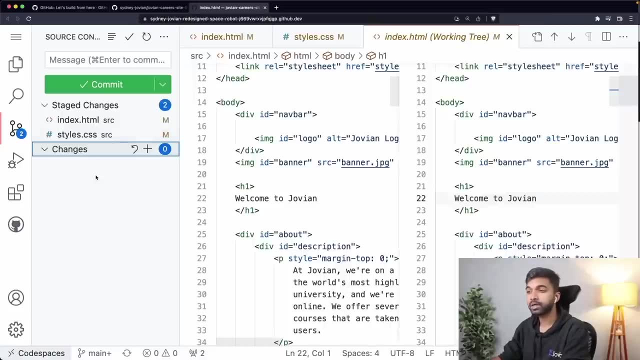 just stage this and let me stage this, or I can also stage them both together by using this single plus button. Okay, Now you can see that we have a couple of stage changes and no other changes. no unstaged changes. So internally, VS code is simply running these git commands for us so that we don't have to. 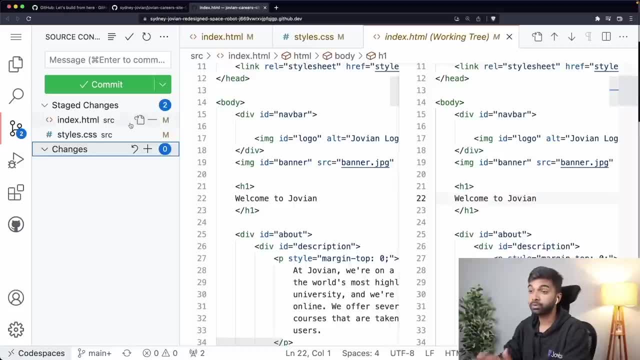 run them, but you should be still familiar with git commands. in case you don't have the sidebar or you're able to, you're not using VS code, Okay. So now that the changes are staged, we can type a message here. So let's say, updated index and styles. 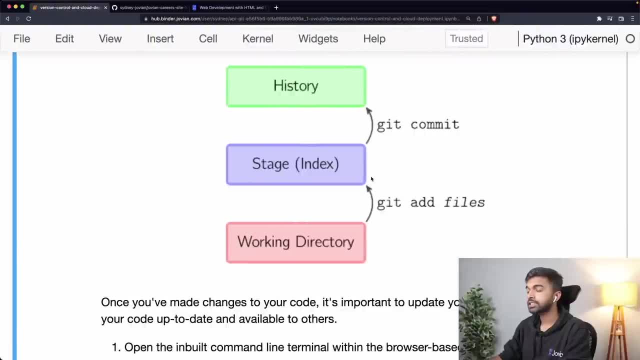 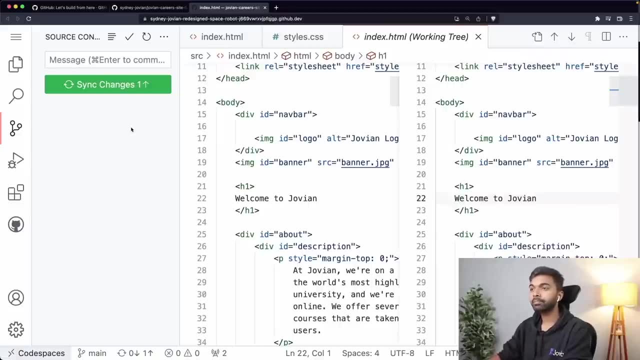 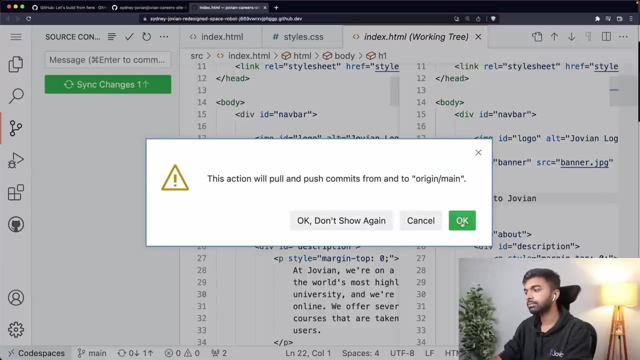 And now we can click commit. Okay, Now the changes have been committed. So we've added the files, and now we've committed the files. but now we still have to send these back to GitHub. So now we can click sync changes. And now it says: this will pull and push commits from into origin main. 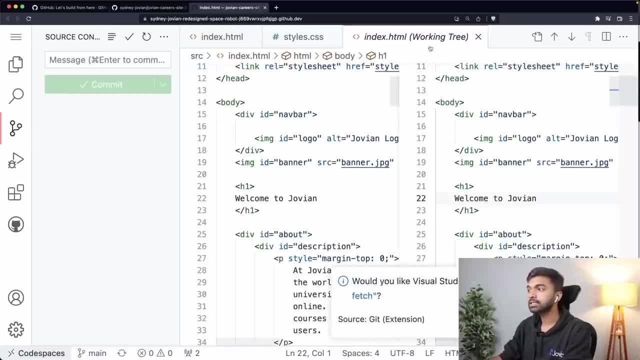 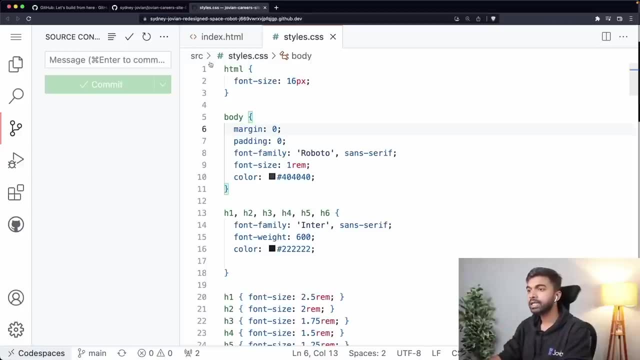 And I'm just going to say, okay, And now my changes are going to be sent up completely Okay. So that is the other way to send updates to GitHub: make some changes, come here, then stage those changes And then commit those changes with a message and finally press the sync button. 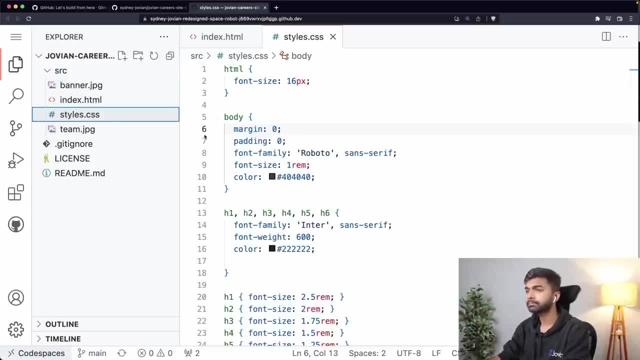 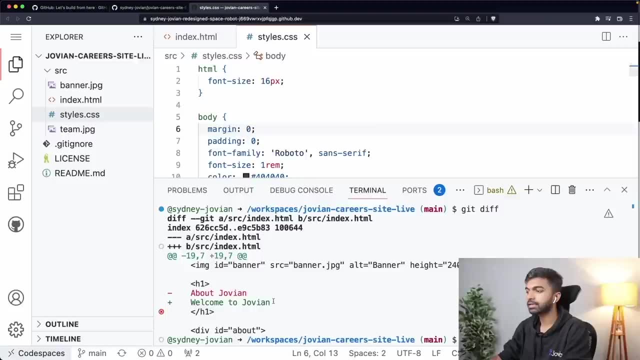 And that is going to push the changes up to GitHub. All right, So two ways to do it. I generally prefer doing it from the terminal, just so that I can keep getting some practice. So I prefer doing it from here on the terminal, but feel free to use the user interface as. 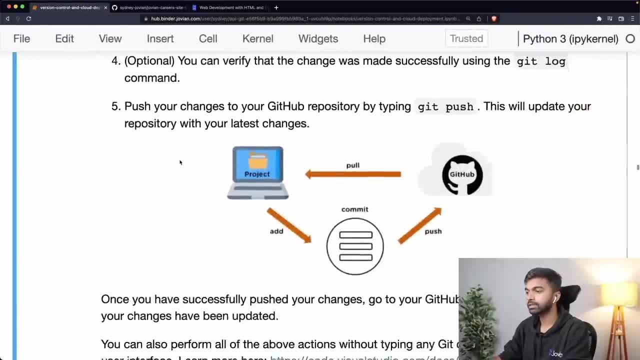 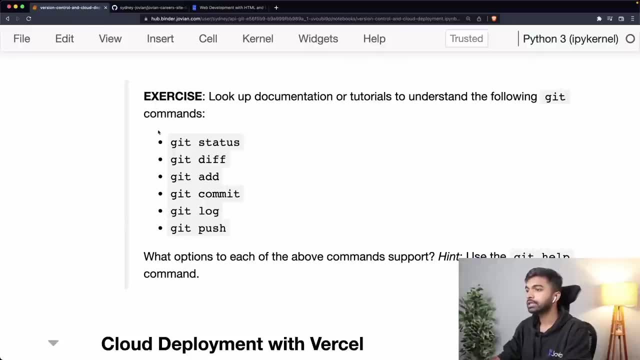 well, Both are equally good enough. Both do exactly the same thing. Okay, So as an exercise, I encourage you to look up the documentation or look up some tutorials, But the most important thing is to understand these Git commands: Git status, which tells: 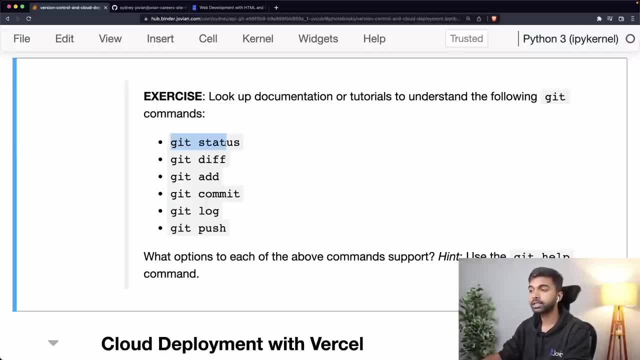 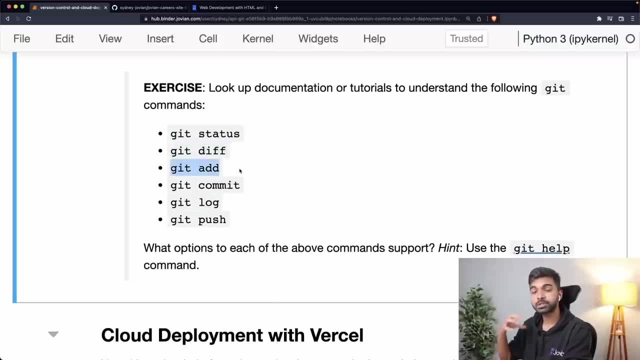 you what untracked files you have, or what are the files with some changes. Git diff, which shows you what are the exact changes in each of the files. Git add, which can be used to stage your files. So go from the working directory to the staging area and you can add individual files or you. 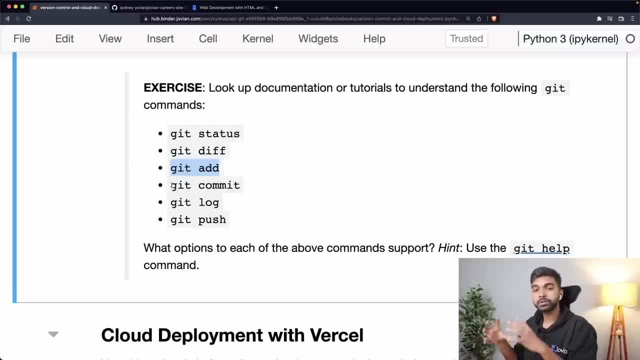 can add all files or you can add a folder at once. Then Git commit, which is used to actually record a new version, then Git log, which is to see the history of commits that you have, and finally git push to push these changes to the remote server or origin. 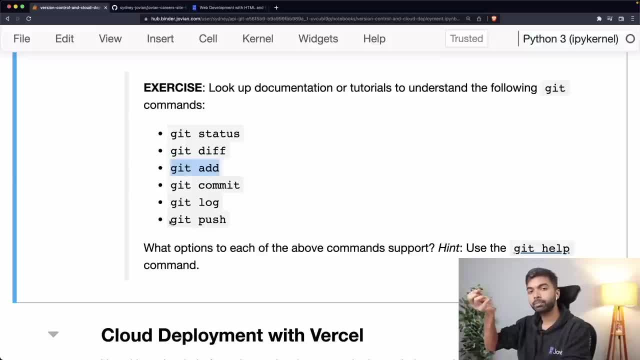 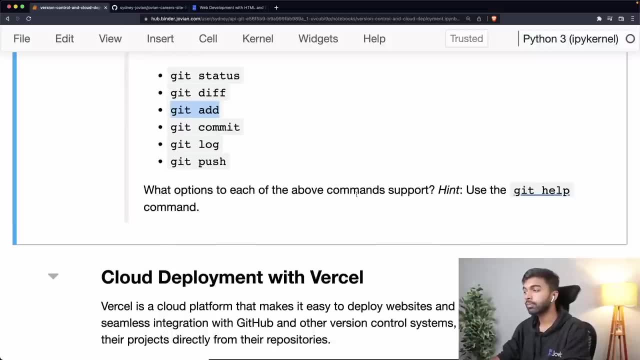 server and you also have git pull in which, which is used to pull the changes from the origin server in case somebody else has pushed some new changes now. all of these commands also support some options, so you can check out some what their options online and you can also use git help. but the thing with git is: 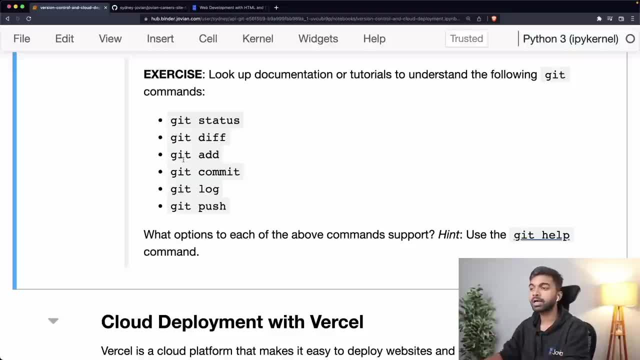 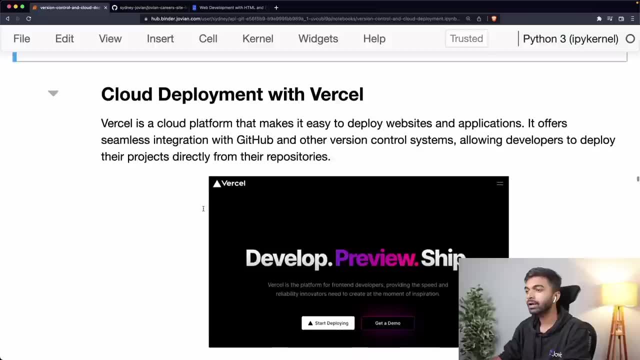 you have to practice, you have to try these out a few times, you have to get stuck a few times and only then you start to feel comfortable. but we've already covered six git terms and there are a lot more that are going to come. but at this point I want to switch gears and talk a little bit about cloud. 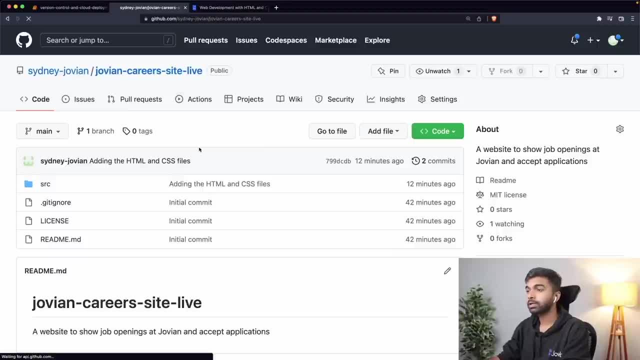 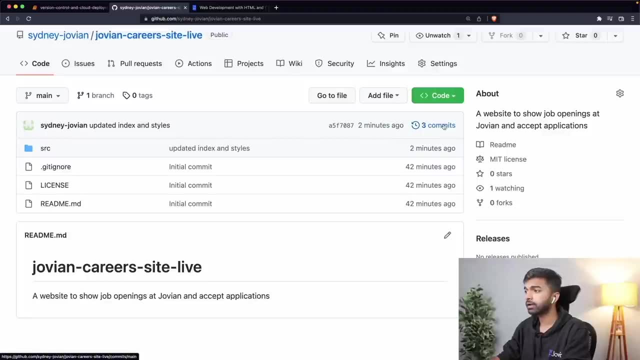 deployment. now we have our Jovian career site live. you can see here that we can see- we can see its history- that three commits have been made so far on github. we can see that there's an SRC folder and that was recently updated with the index and styles that we committed directly from vs code and there are some. 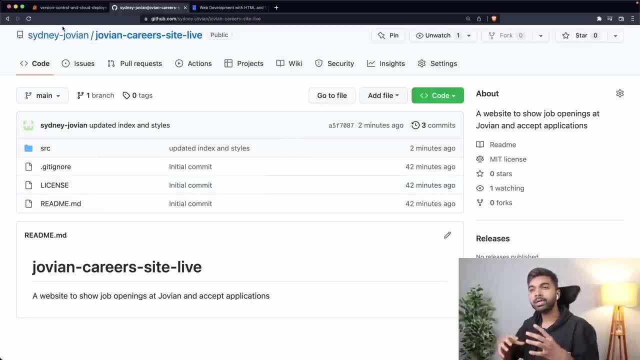 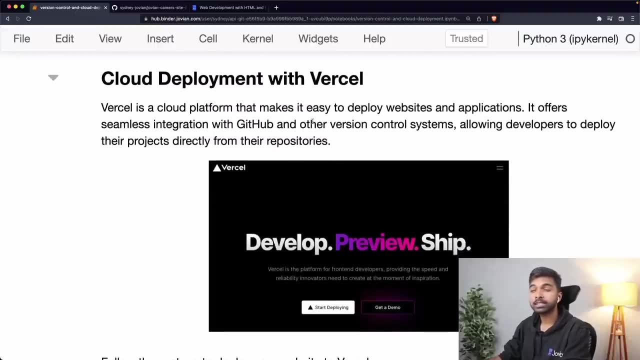 other files from the initial commit. how do we get to the github file? and how do we get to the github file and how do we take this and how do we easily deploy it to the cloud? we're going to do that using this platform called Vercel. Vercel is a cloud platform that makes it really 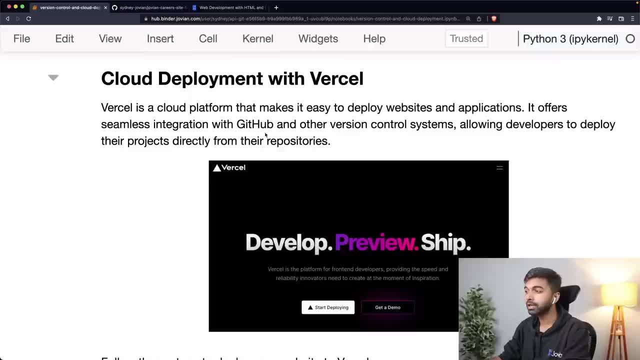 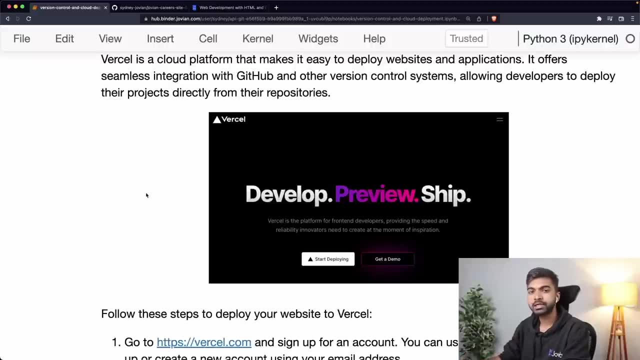 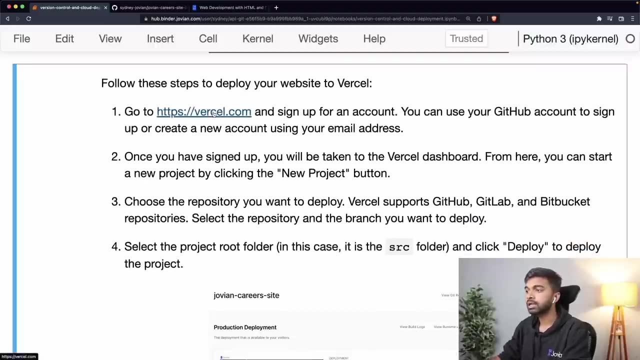 easy to deploy websites and applications, and it offers a seamless integration with github and other version control systems, allowing developers to deploy their projects, almost seem almost instantly, without any additional coding or any additional work. so here is what we are going to do: we are going to sign. 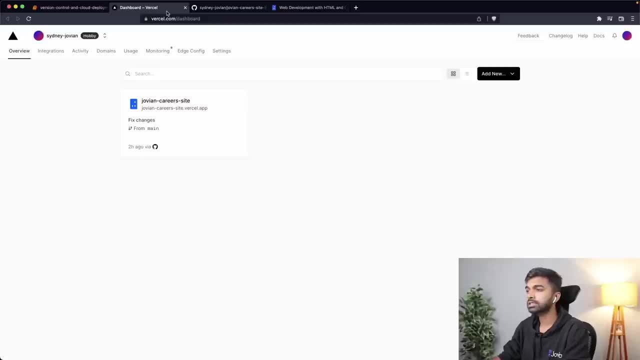 up on verse L dot-com, so let me just sign up. in case you're not signed up on already, you'll need to sign up. I am already signed up and signed in, So I'm good to go. Then you will be taken to the Vercel dashboard as soon as you sign up. let me zoom in here. 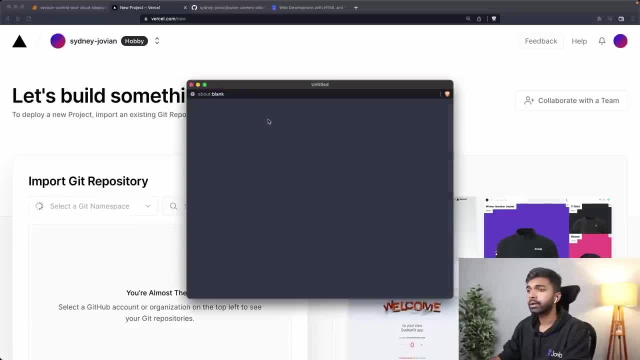 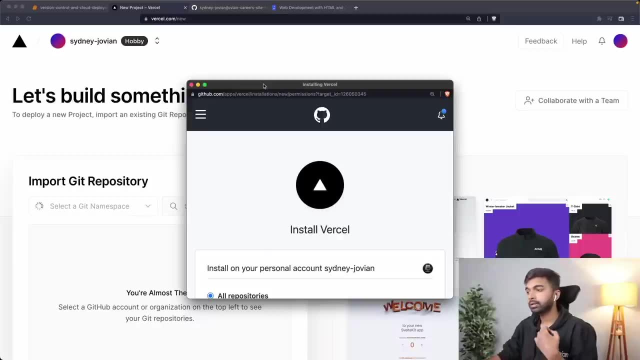 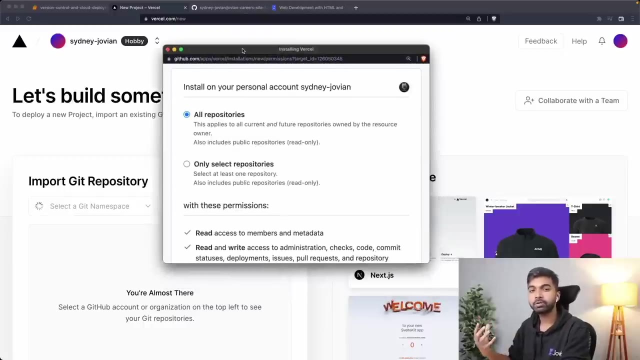 And you can add a new project. So I'm going to select new project. And when I select new project, it is going to ask me access for my GitHub repositories. So once one, when you're signing up, try to sign up with GitHub so that you can give permission to sign up using. 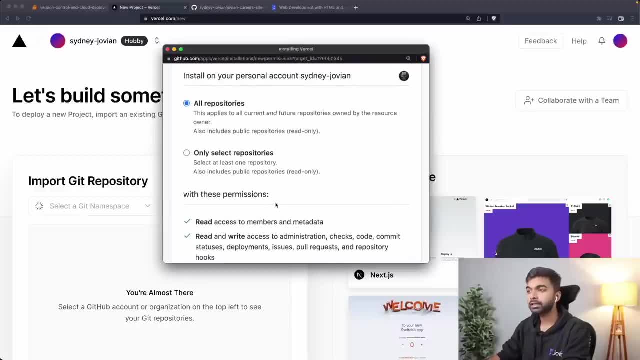 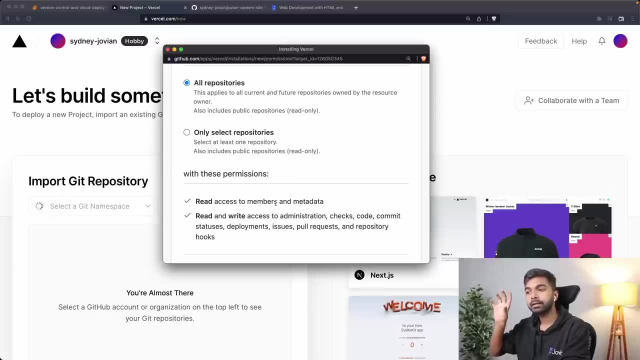 GitHub directly. But second, when you actually try to create a project, Vercel is going to need access to your GitHub repository so that it can, it can pull out the code And it can then deploy them to the cloud- not just public repositories, but also private repositories. So you can either 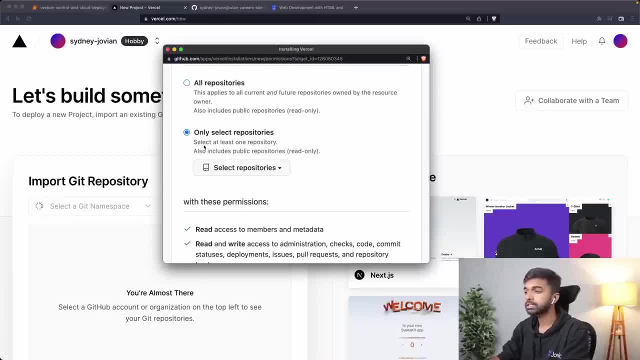 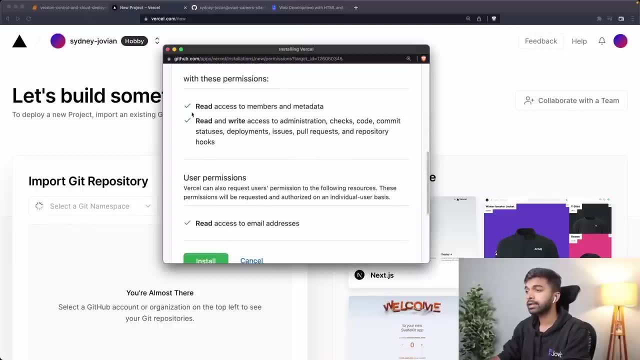 give access to all repositories or you can give access only to select repositories, And you can select which repositories you want to give access to. In my case, I'm going to give access to all repositories And it is going to have access to read and write because it is also going to write. 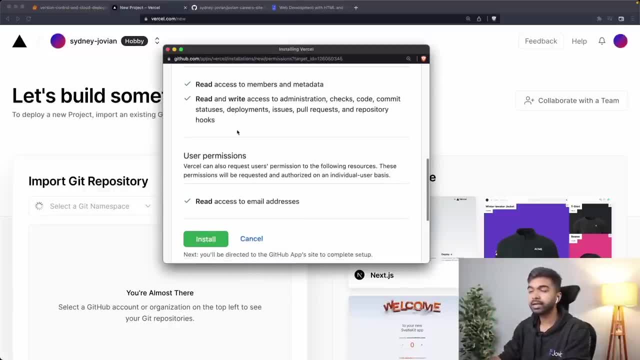 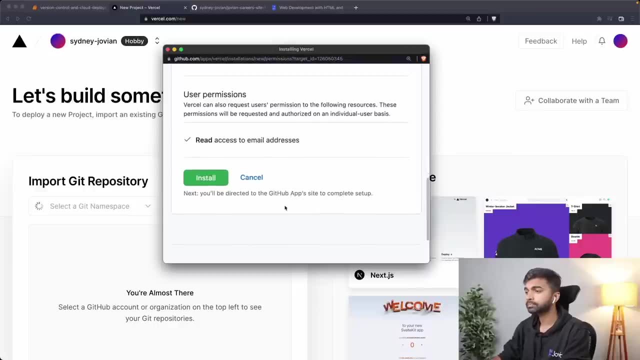 something into your pull request, which we'll talk about later, But in general, yeah, you need to give Vercel full access to your code so that it can pick it up- even private code- and deploy it to the cloud. Okay, now let's click Install. So that is going to install the Vercel GitHub application. 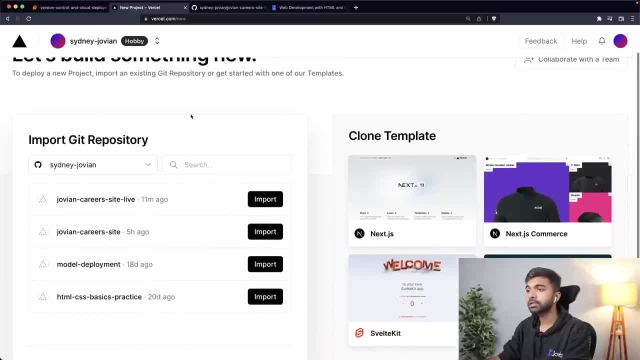 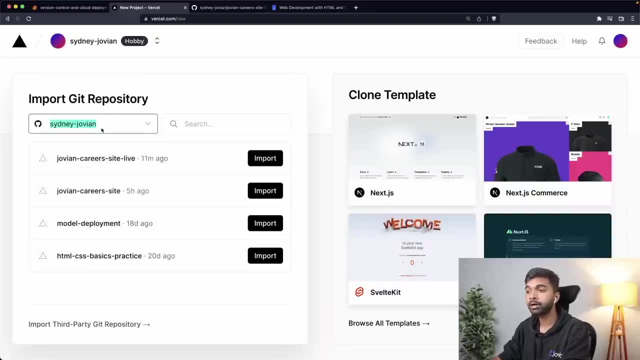 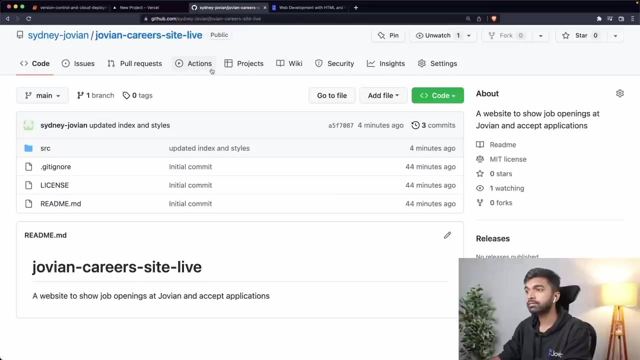 essentially. And now, at this point, you will see this new project box, And in this new project box you can select which GitHub account to use, in case you've connected multiple GitHub accounts, And from that GitHub account you can select which site you want to actually deploy. So I am. so. my repository is called Jovian career site live. 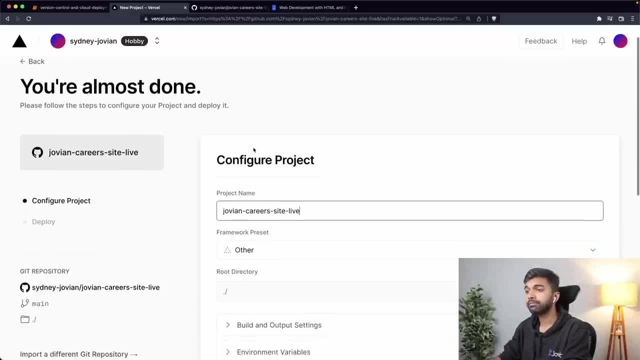 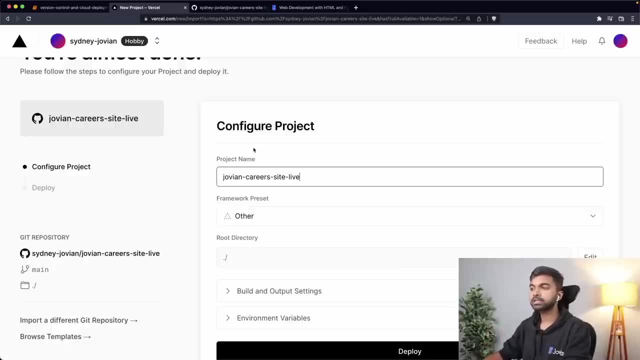 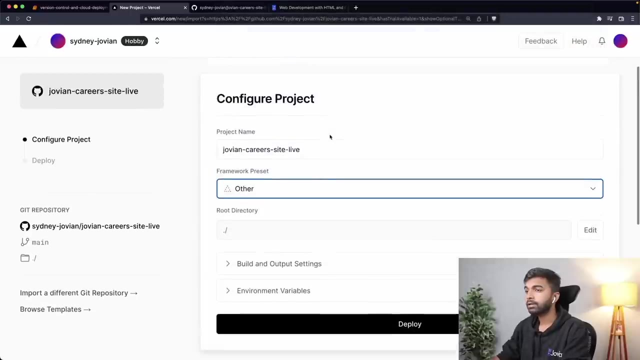 So I'm just going to click import Jovian career site live, And now I have to configure the project, because Vercel has configurations for all kinds of various different projects. So you can see here that it has a bunch of different pre configured frameworks, And first you can set a project name. 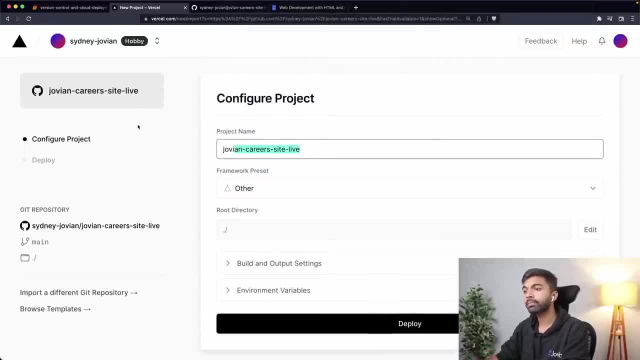 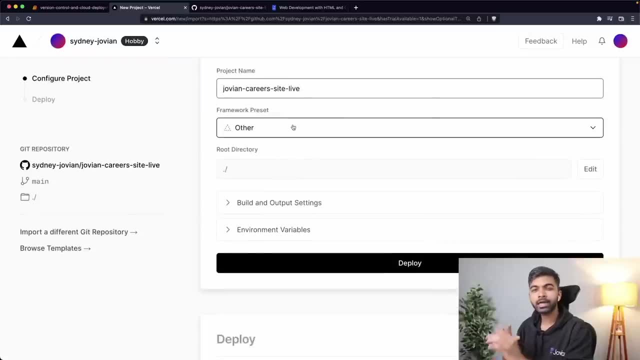 I'm just going to keep the project name on Vercel the same As the project name on GitHub. no change here. So Jovian career site. live the framework preset. I'm going to select other because I'm not actually using a framework. 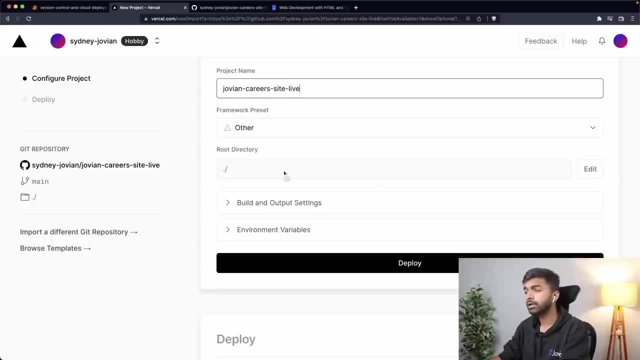 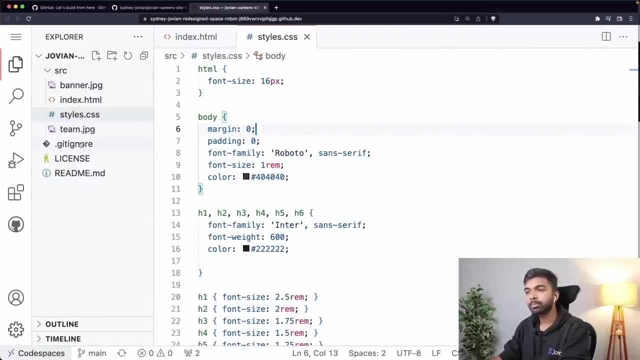 I'm just using simple HTML and CSS files. then I need to select the root directory which needs to be deployed. So remember, we created this SRC directory. we don't want to deploy our gitignore file and license and readmemd. That's not something we want to put on. 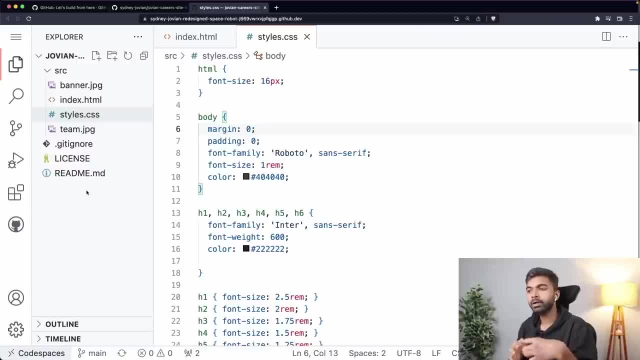 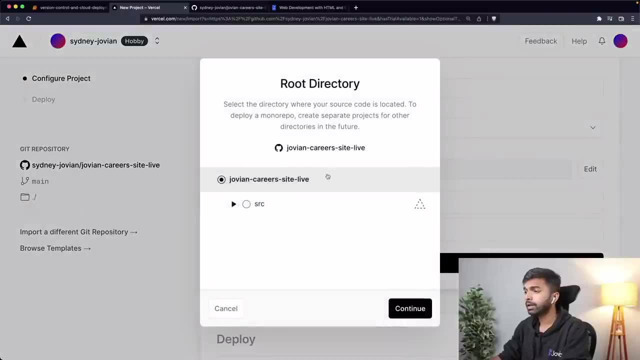 the website itself. That's something that we want to just put on GitHub. So let's select the SRC from the SSC directory as the root directory. I'm going to click Edit here And I'm going to just select the SRC directory as the root directory and click Continue. So we are. 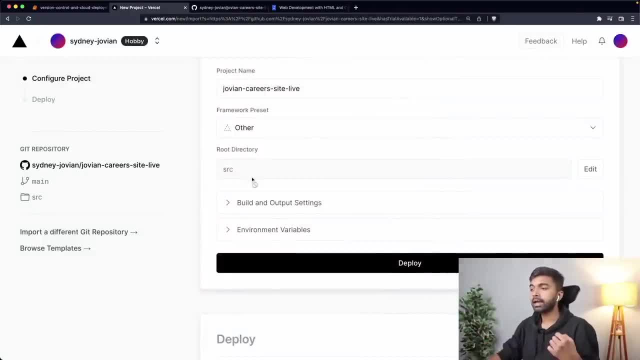 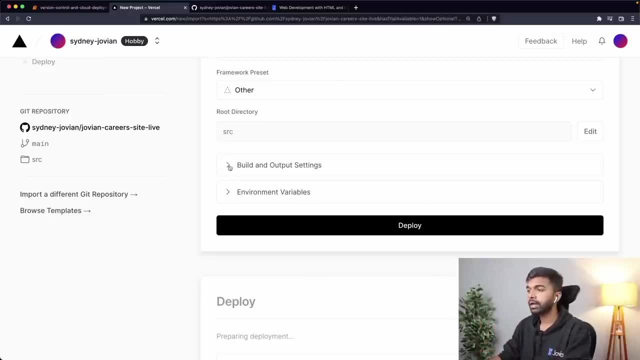 telling was so that we have a simple website, no framework, and we are simply going to pick the code from the SRC directory and just directly deploy it to the cloud, And there are other settings which we don't need right now, So I'm just going to click Deploy. 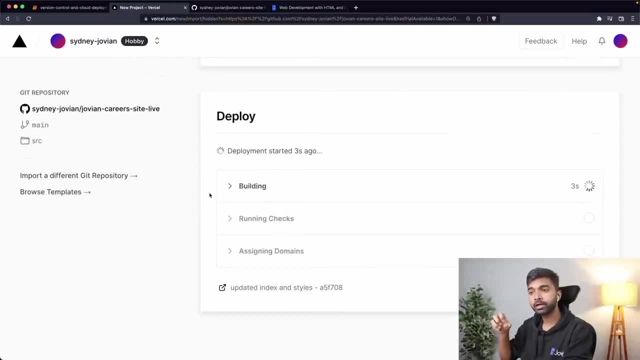 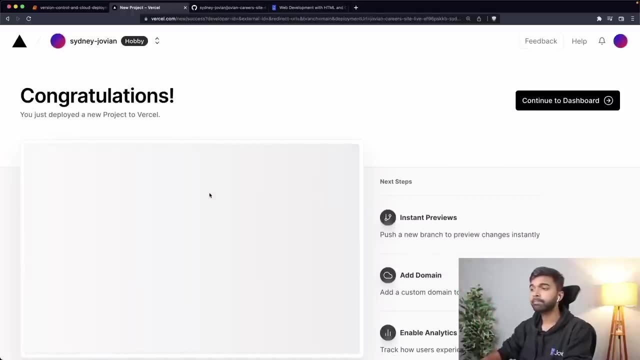 Now, as soon as we click, deploy was so, let's pull it out, all the code from our GitHub repository. it set up a machine on the cloud, conceptually speaking, and it has deployed the code, and you can see here that this is what the deployed site looks like. okay, you can actually click continue. 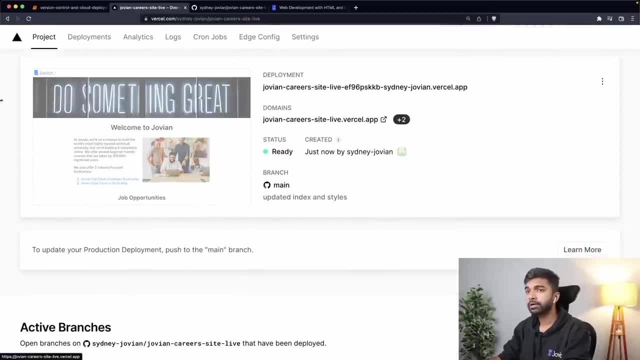 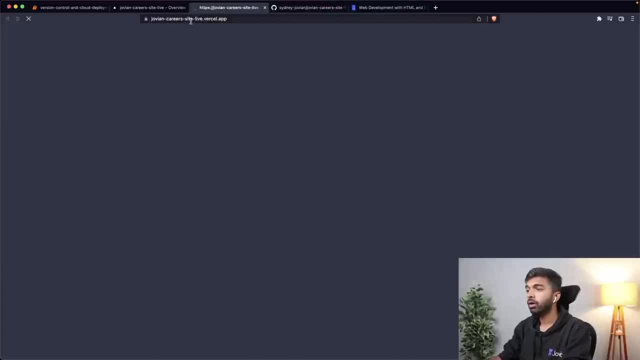 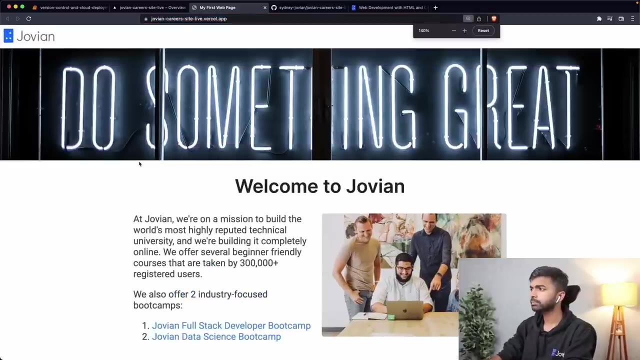 to dashboard and here you can see that we have a preview of what the deployed site looks like and we also have links to a couple of deployments. so by default your project name dot- vercel dot app is the location of the deployed website. let me just zoom in here so you can see. now we have 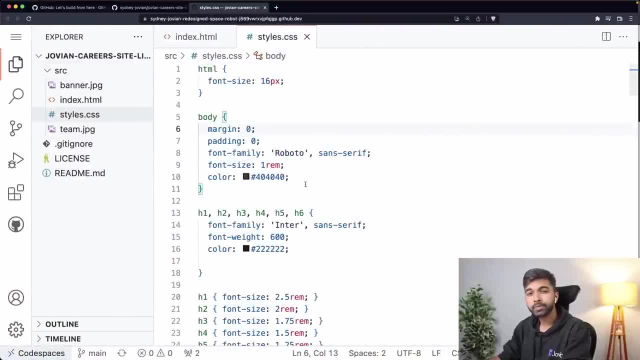 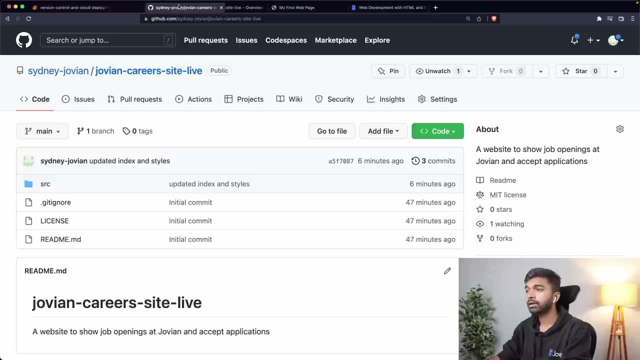 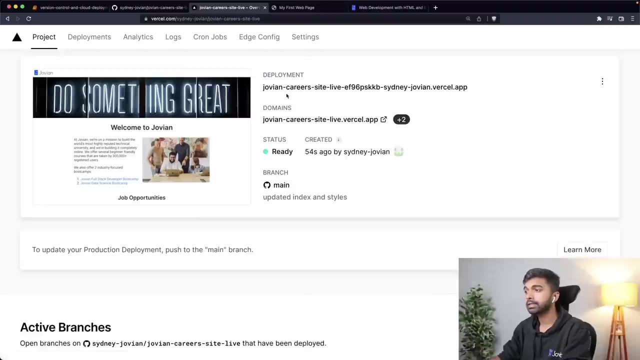 deployed our website. so now we are developing on GitHub code spaces and we are pushing our changes back to GitHub. and then we are. we have connected our GitHub repository to vercel and vercel is picking up the GitHub repository, the main branch, and it is deploying it automatically, right you? 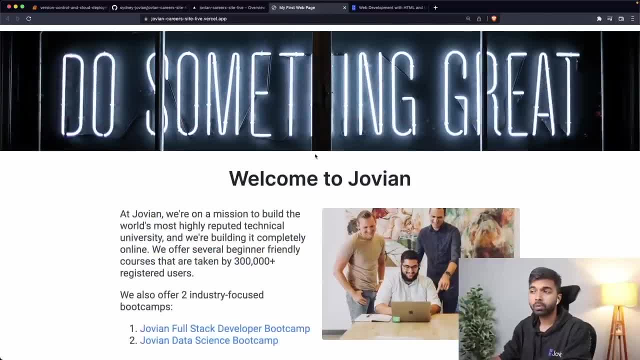 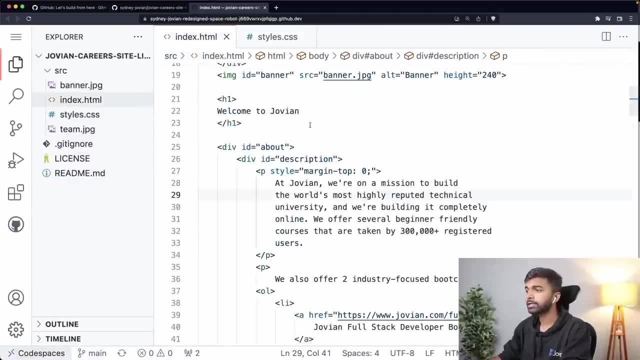 can see here that it is deployed automatically. so that is how easy it is to deploy, and the next thing you can do is anytime you make a change. let me come back here in indexhtml and let me just change this to about jovian, and I'm just going. 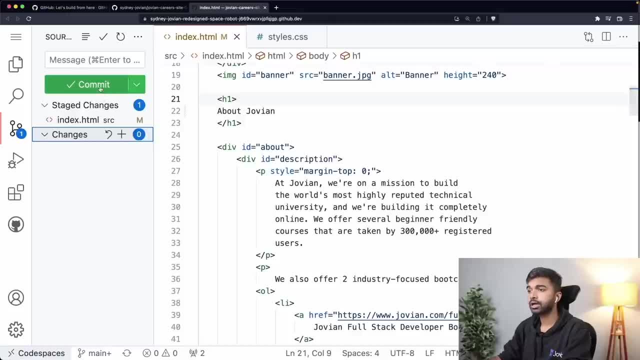 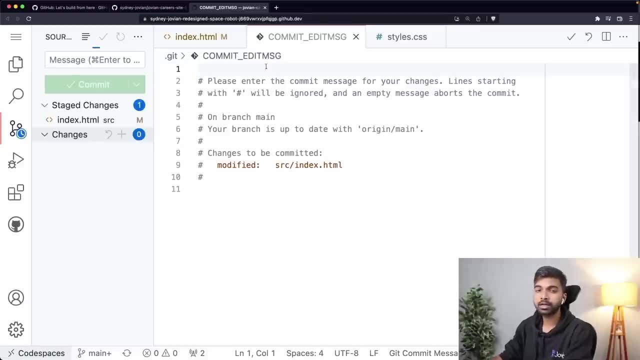 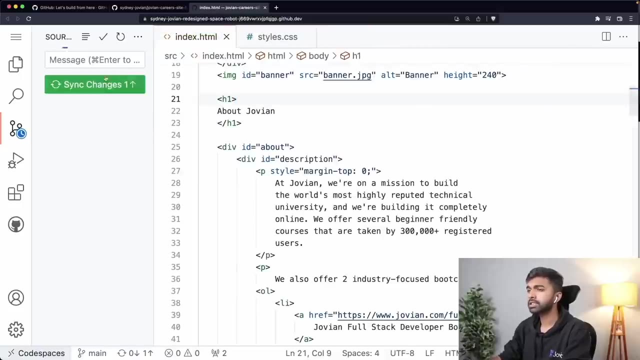 to make a quick commit here. so I'm going to stage the change I am going to commit and sometimes when I when I try to commit without a message, it will ask me to put in a commit message. so let me just say change to about jovian and let me close that. so now it is committed, now I am going to push again and 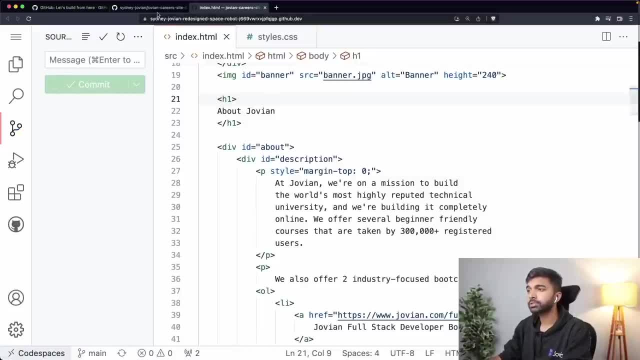 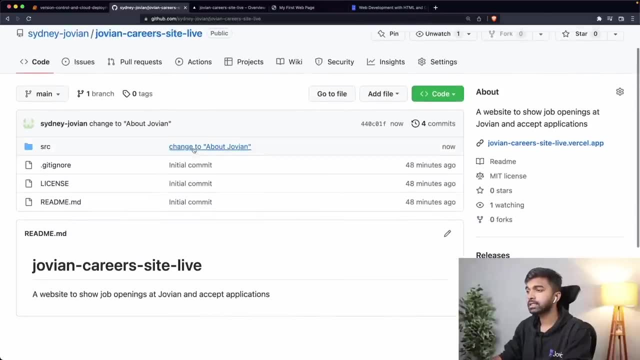 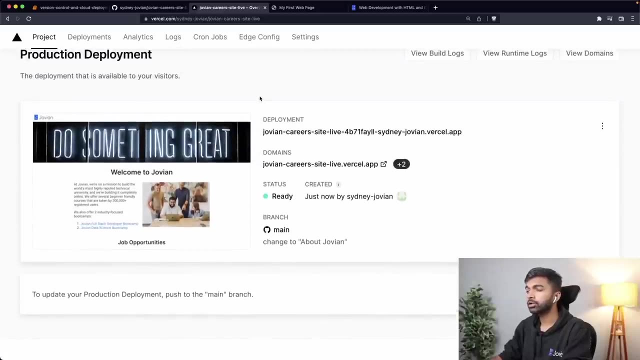 okay, let's push it. so now the changes are going to get pushed. so now the changes are pushed. here to joven Career Site Life, you can see that we just changed to avoid jovian. and once you push, what happens is you can see that a new deployment is going to be made by vercel automatically. 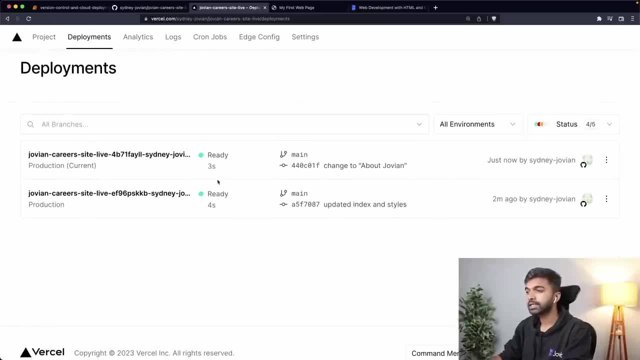 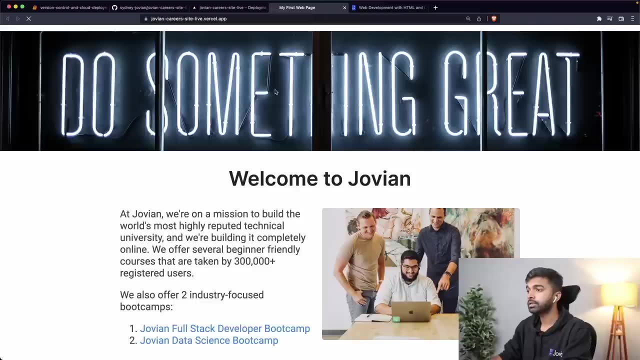 so you can actually see a history of, actually see a history of deployments. You can see, just three seconds ago a new deployment was made and this new deployment was made on the commit change to avoid about Jovian. So on, Vercel, welcome to Jovian. changes to about you. So anytime you make any changes to your GitHub repository and push the main branch or you make changes on code spaces, push the main branch to GitHub. Vercel automatically picks up the new change from the main branch and automatically redeploys it. 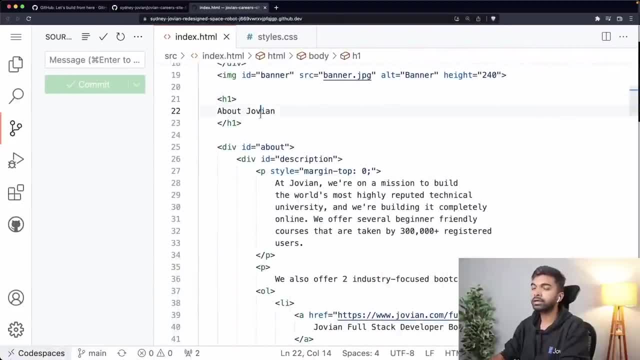 Isn't that nice That all you have to do is just go on coding here and keep checking your live preview. whenever you're ready, You can just go in and you can just add all your changes, commit them and push them, And once they are pushed, Vercel will pick them up and deploy them. 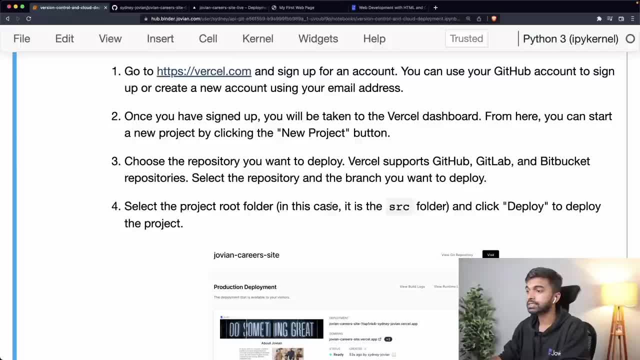 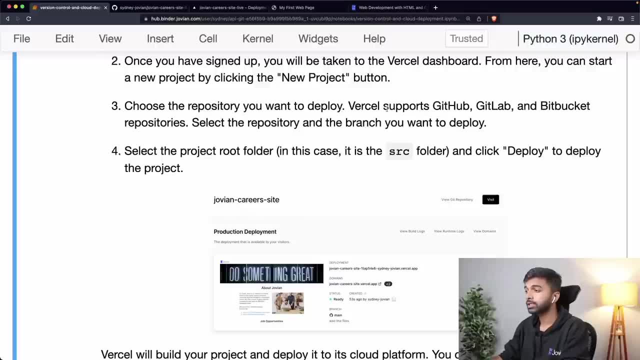 And that is a deployment workflow that you are going to work with, more or less. So you go to Vercelcom, sign up for an account. Once you sign up, you create a new project and you choose the repository that you want to deploy. 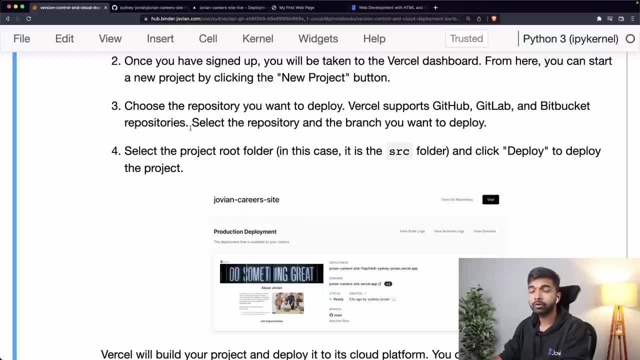 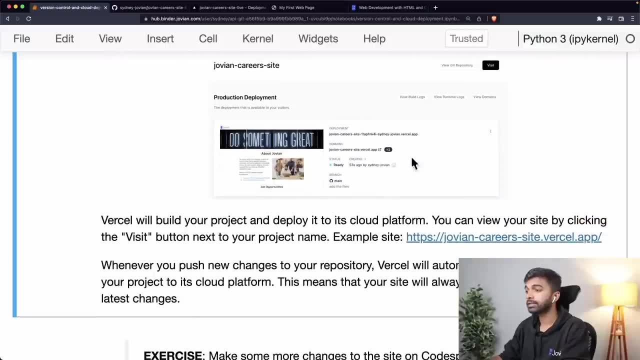 It supports GitHub, GitLab and Bitbucket and you'll have to connect and give access to Vercel. then you choose the project root folder- In this case it is the SRC folder- And then you click deploy and then it creates a deployment. 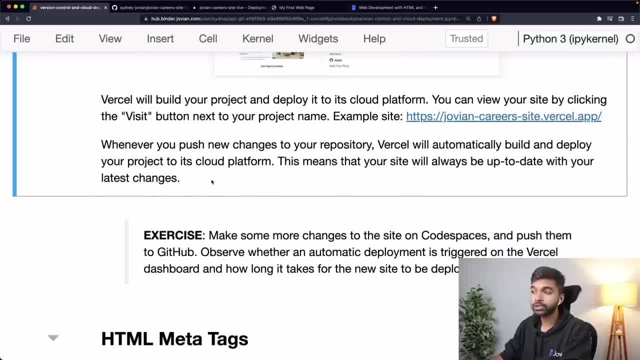 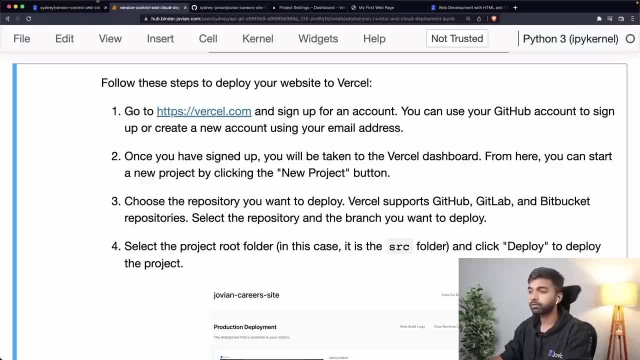 So it builds your project, deploys to the cloud, And whenever you push new changes to your repository, especially the main branch, Vercel will automatically build and deploy your project. So that creates a very nice workflow. Now, one of the goals in the problem statement was to add some meta tags and 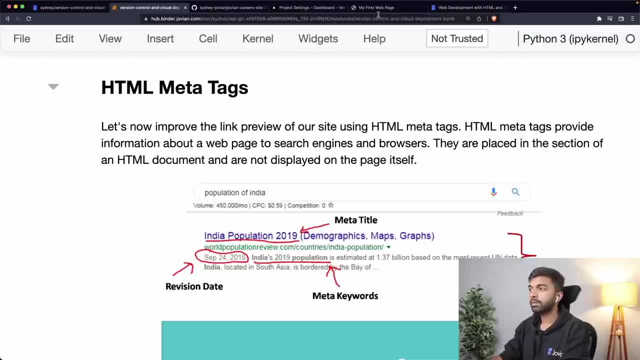 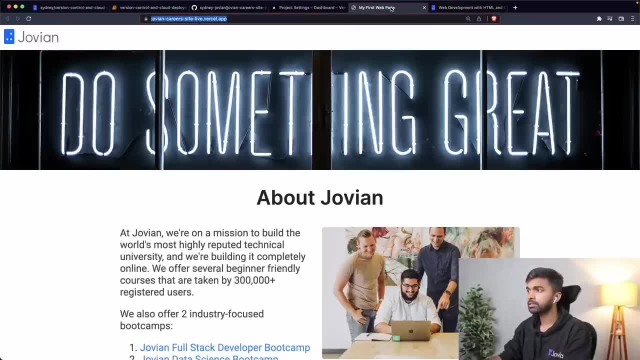 improve the reviews of this webpage. So now we have this Jovian careers sitelifeVercelapp. But one thing you'll see here is, if I zoom in a little bit here, you, you see, you see it says my first webpage at the top here and it also doesn't have 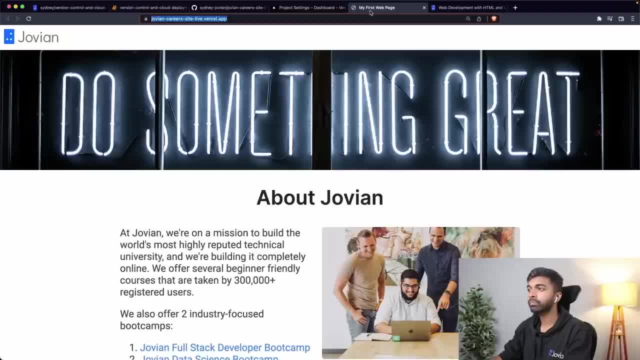 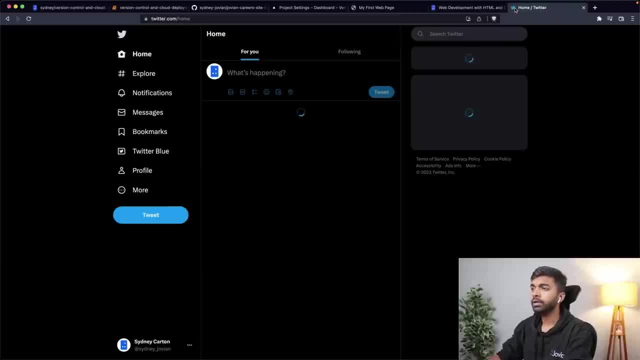 an icon, so it would be nice to maybe get a Jovian icon in here as well. Another thing that you can check is if you try to share this on LinkedIn or Twitter or elsewhere. it's not going to show a nice preview. 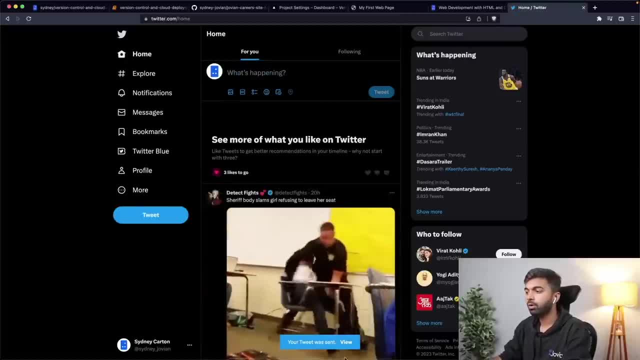 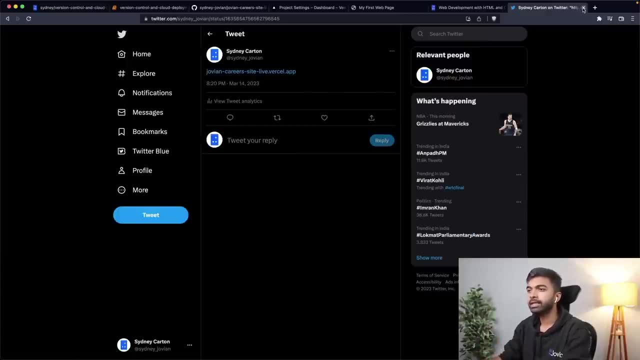 Okay, Normally, when. normally we expect to see a nice preview of our- Yeah, normally we expect to see a nice preview of any website that we share on the internet- but that is not showing up. So normally what happens is when, when a website is found by Google, or when a 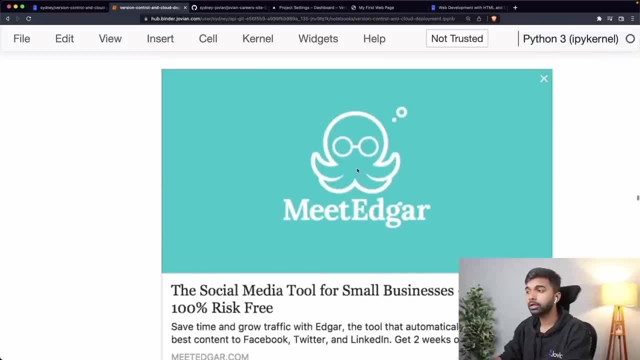 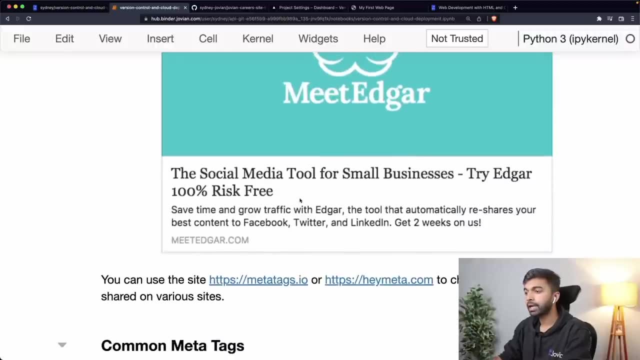 website is shared on, let's say, LinkedIn or Twitter or Facebook, they automatically pick up this preview image. There's something that can be configured and they automatically pick up maybe a title and a description, all of this. So where does this come from? 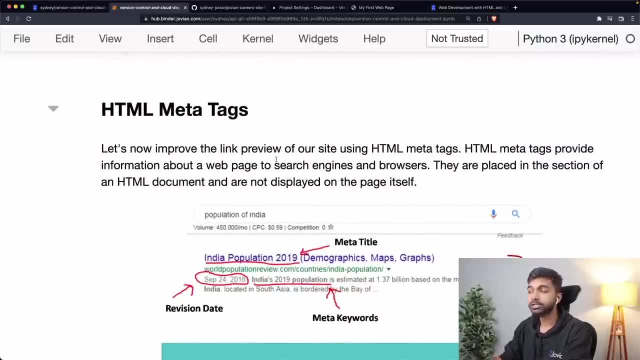 Well, all of this is done using some Special Tags, special HTML tags called meta tags. HTML meta tags provide information about a webpage to search engines and browsers, and they are placed in the head section of a HTML document and they're not displayed on the page itself. 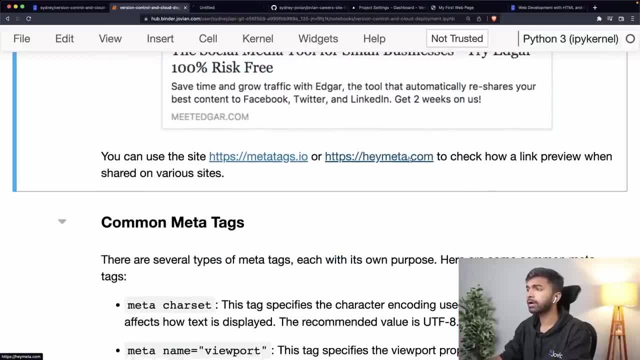 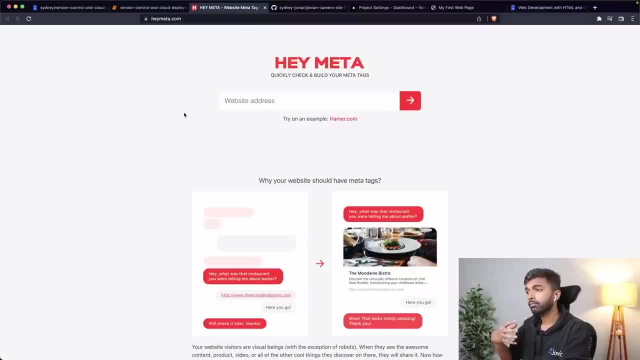 So you can actually use a platform like heymetacom. You have these tools like heymetacom to actually check what the preview for a particular webpage is going to look like. So let's say, if I just copy this, my first webpage link. 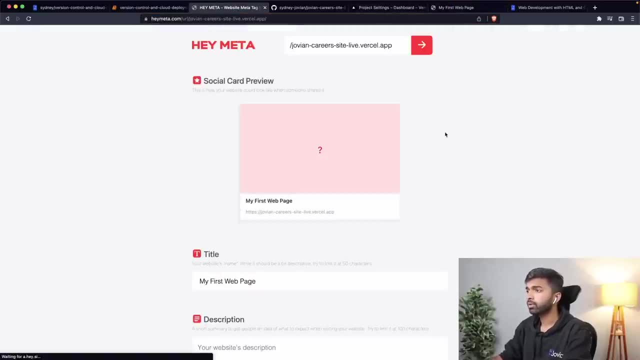 And put it here and I check what the preview is going to look like. So you can see here that there is no preview image and the title of the webpage is simply my first webpage, which is not very informative, and there is no description as well. 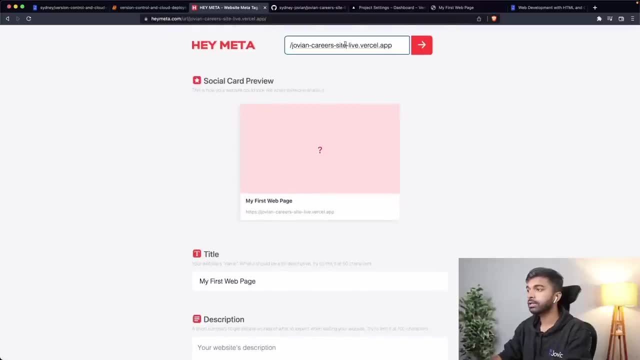 So there's no description, There is no image, none of that. on the other hand, most modern websites, So let's say, wwwjoviancom. If you share this link with somebody on social platforms, or maybe just check on heymetacom, you'll see this preview image. 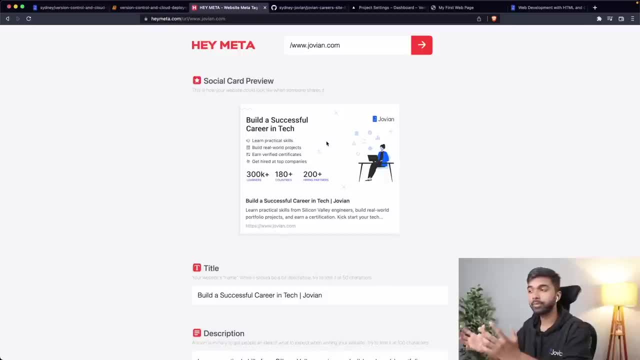 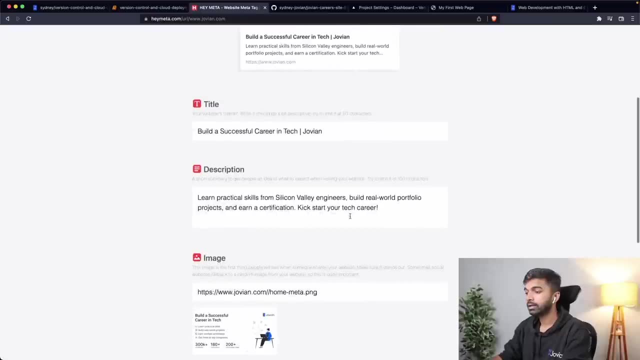 It says: build a successful career in Trek. This is not there anywhere on the actual page, but this is just for the purpose of preview, and you will see that it has a nice title and it has a nice description as well. So all of that is something that is going to show up automatically. 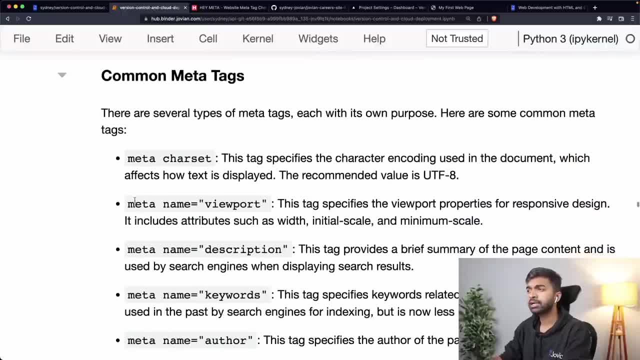 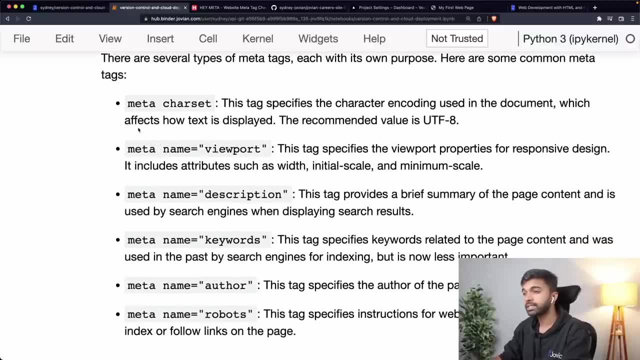 So all of this is achieved using meta tags. So there are several types of meta tags, each with its own purpose. So here are some of the more common meta tags that will be used in most webpages. There's something called a meta-carset. this is used to inform the browser. 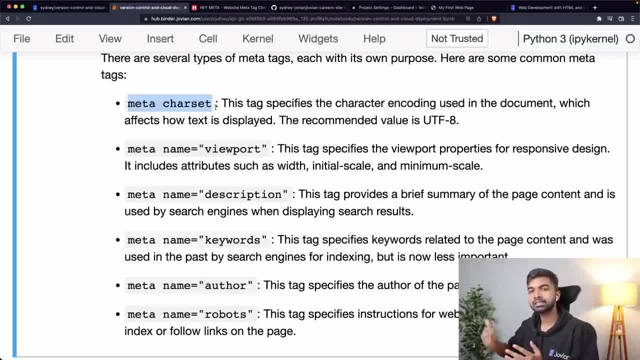 There are several character sets. There's something called ASCII, something called UTF, et cetera. So what is the character encoding that this page is using? So this is often something that is set to UTF-8.. Then there is something called the viewport meta tag. 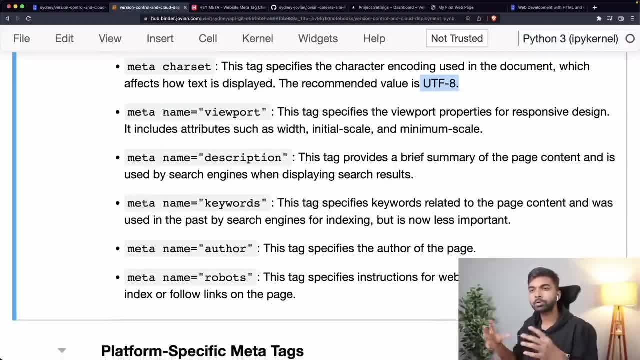 This is used to inform the browser how to scale up or down, how to zoom in or out the website on a mobile screen. Again, there is a standard value that is preferred for more modern websites. Then there is this meta name description. 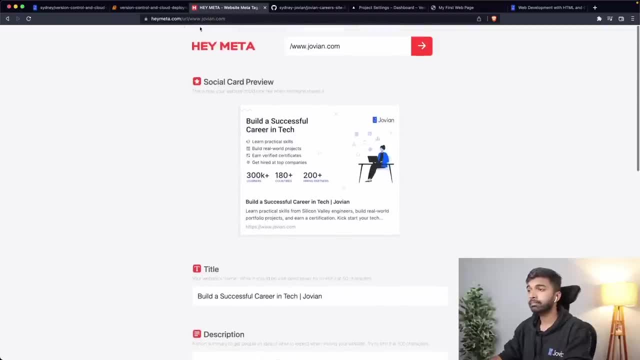 And this description is actually picked up by platforms when you share this link, when you share the website as a link, So the description is not actually shown on the page, but it is just picked up as a preview by Google. And whenever you share the platform elsewhere, you can also set a meta. 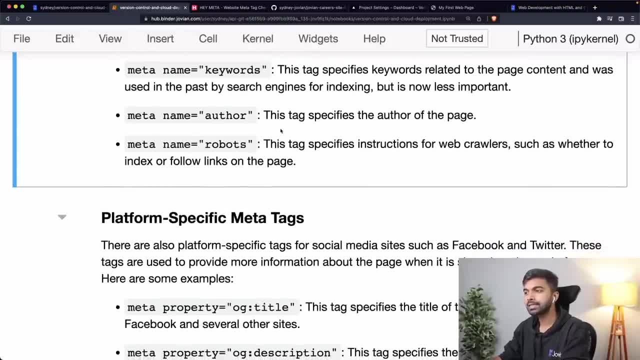 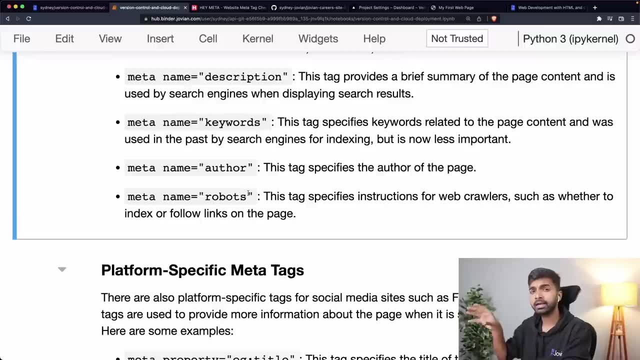 author- not particularly useful these days- And you can also set meta keywords and meta robots. Meta robots provide some instructions whether search engines should index this page or not, And meta keywords is used to specify some keywords that are that were used in the past for search engine indexing but are 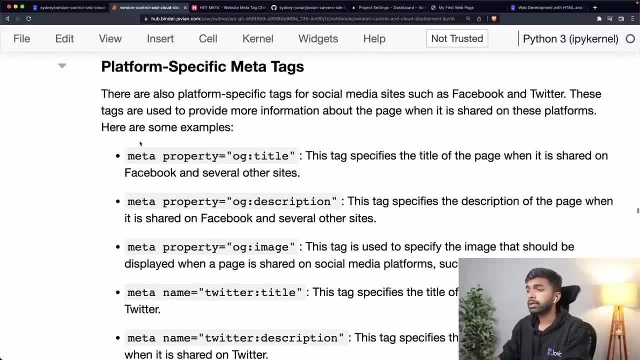 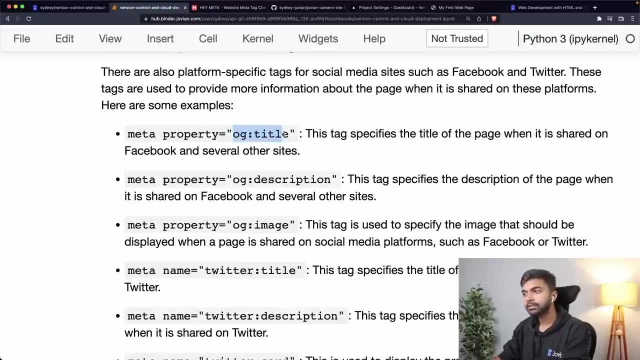 not now very less important. Okay, There are also platform specific meta tags So you can take your URL, your website URL, and make it show a different way on Facebook and a different way on Twitter, for example. So there is this property called OG title. 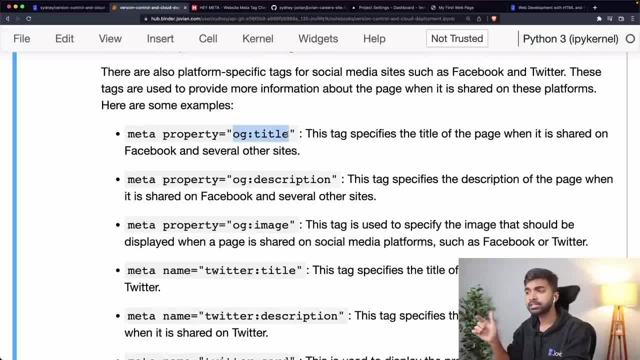 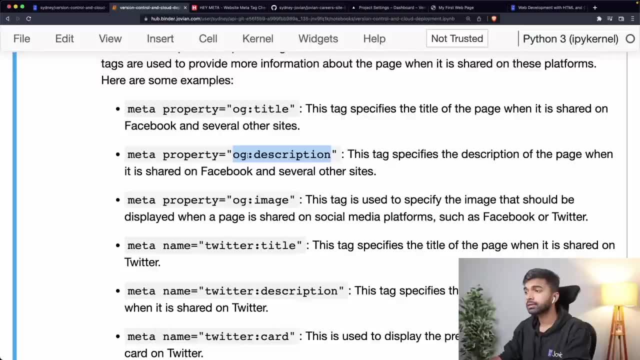 So this is the title that is going to be picked up by Facebook, LinkedIn and several other sites. OG stands for open graph And there is this property called OG description, Which is picked up for description on Facebook. You can also specify this image using OG image. 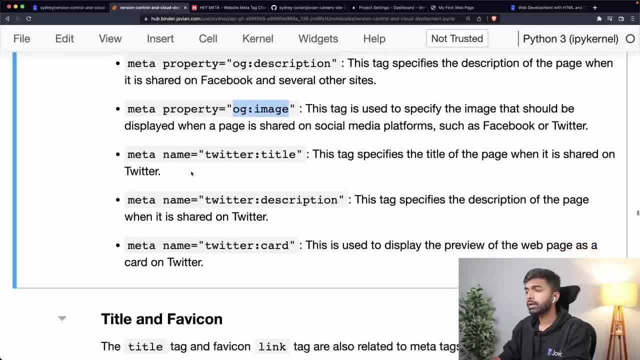 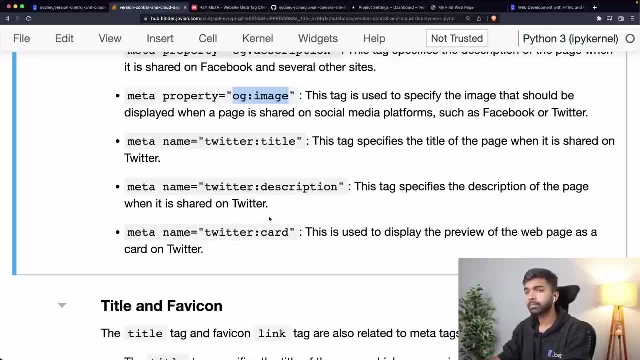 This is the image that shows up here. And, finally, you can specify similar title description and a card setting for Twitter as well. Okay, So those are all the meta tags that you can have on your website, on your webpage, And apart from this, you can also have a title meta tag and a fav icon. 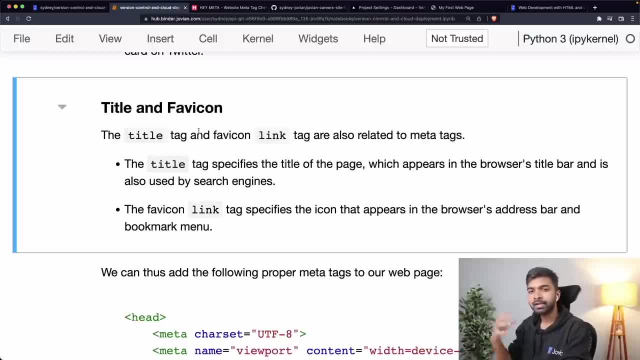 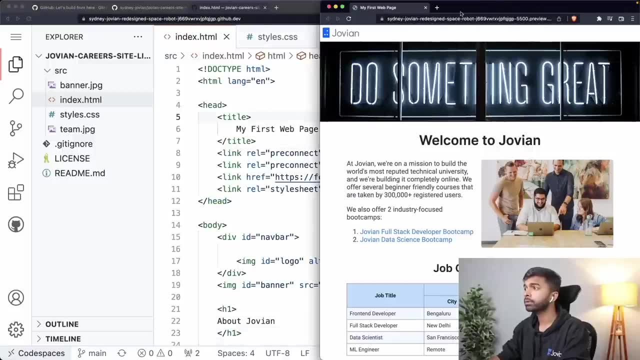 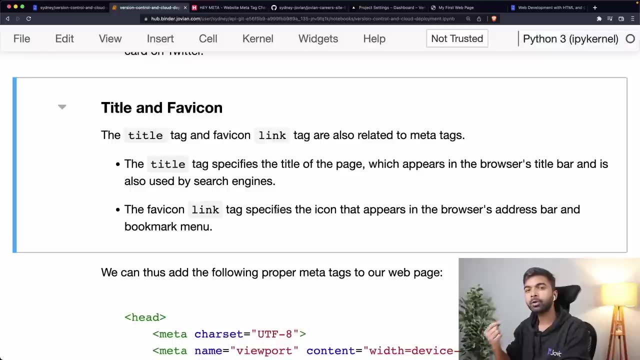 Link tag, So the title. this title is not a meta tag exactly. It is simply used to set the title of the page. So this is also important, because this is what shows up on the browser tab And you have a link, like a link tag, which contains something, a link to. 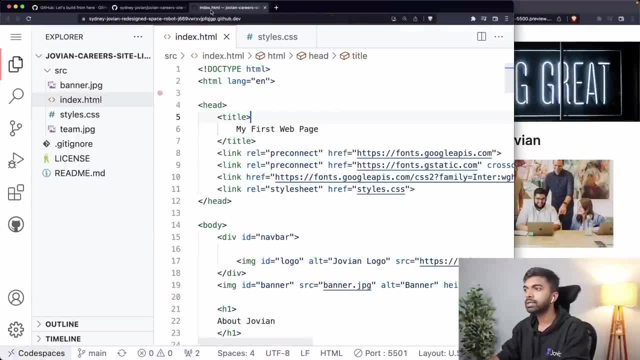 an image called a fav icon, and that image is the image that shows up over here. So right now you're just seeing a small web image here, but instead, let's say, here you have the GitHub logo And That's where you will see the Jovian logo on Jovian. 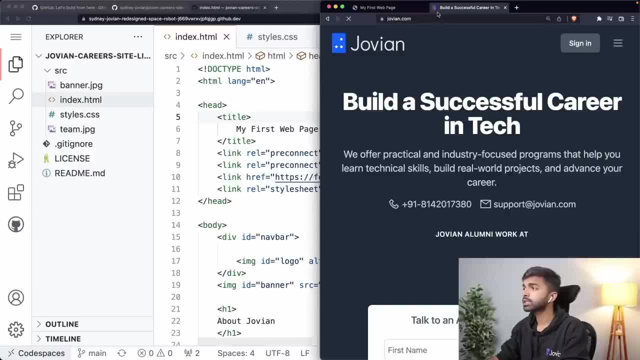 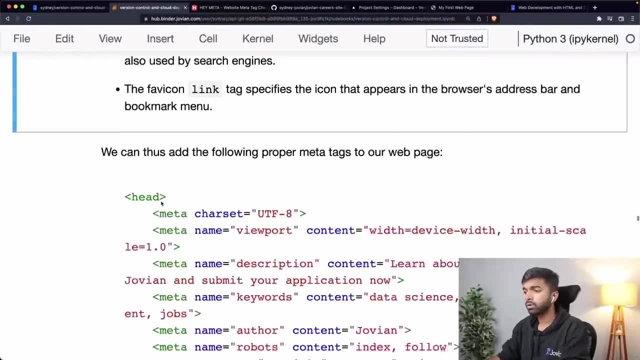 Let's say I open wwwjoviancom, You see the Jovian logo, but putting a logo here in the browser tab is done using the fav icon. Okay, So what we'll do is we'll go ahead and add a bunch of these meta tags to our webpage. 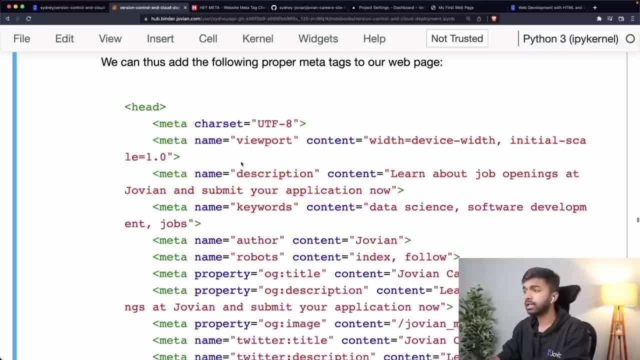 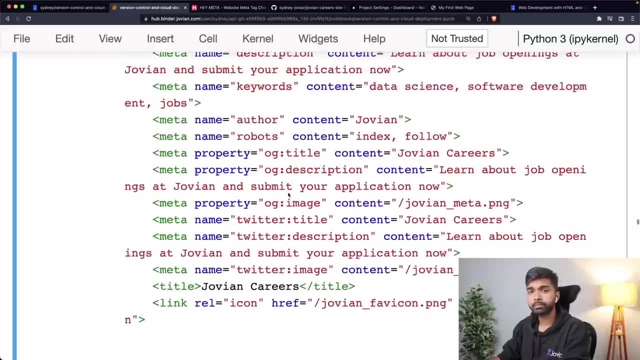 So we can take all of these meta tags. We have car set, UTF, eight, name, viewport, description, keywords, author, robots, et cetera- And we are going to add them all to our project. And, specifically, a couple of images also need to be added. 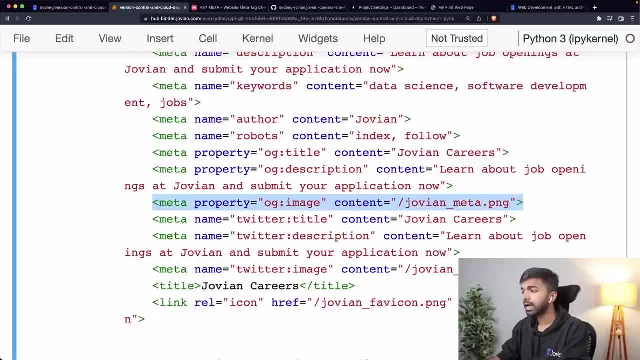 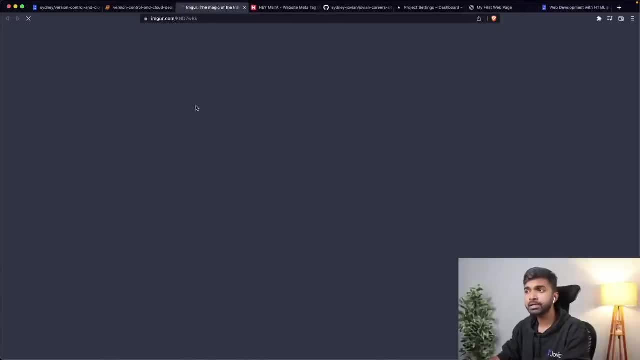 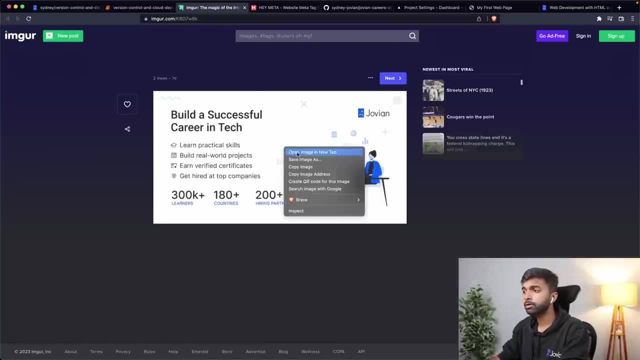 See, we have this one meta tag called OG image and that we are going to set as jovianmetapng, and the file jovianmetapng is here So you can download it in case you want to add it. Yeah, this is the. this is the image that we're going to use as jovianmetapng. 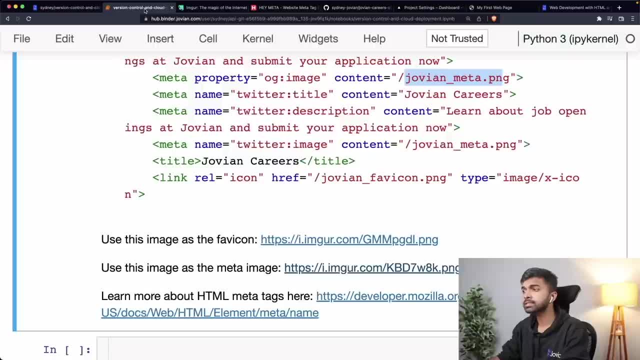 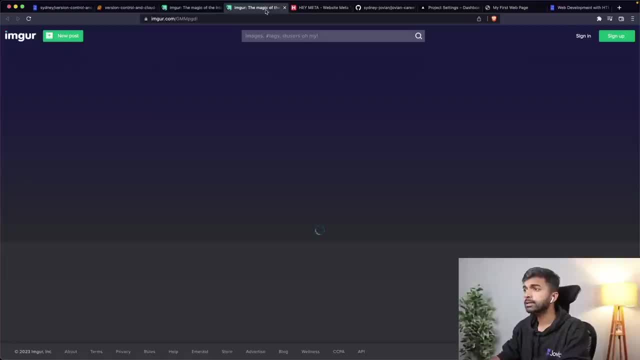 So I can just save this image to my desktop and then upload it to Codespaces, And we also have a meta Yeah Image for a favicon. So this is the favicon that we're going to use. This is the icon that is going to show up on the browser over here. 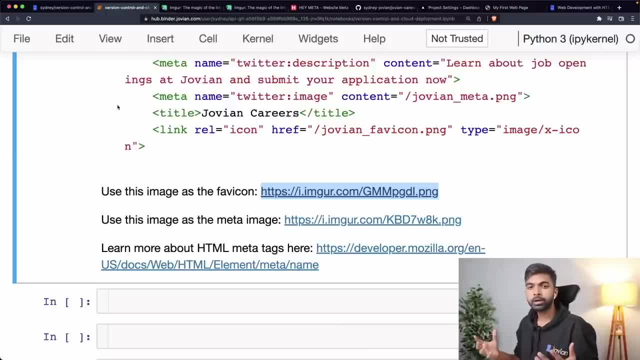 Okay. So again, these are not things that you learn in a introductory HTML course. but to build good, practical, modern websites, you need to have good meta tags. Otherwise your websites are just going to look random on the browser or when people share them. 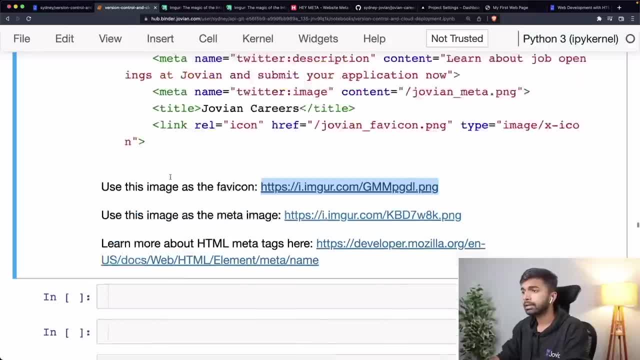 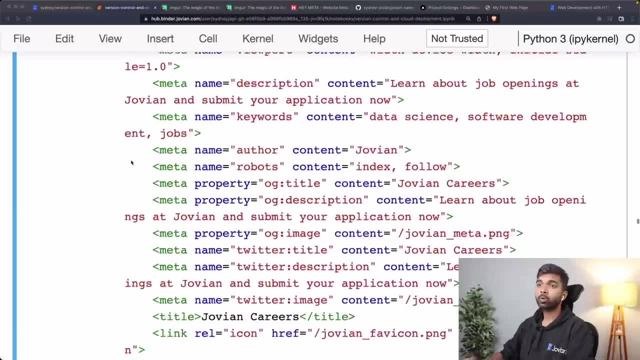 Okay, There's more information you can learn about meta tags here, but these are the tags that we're going to add into our web page, All right, Well, so now we want to add meta tags, So we basically want to add all this code into the head tag of our indexhtml file. 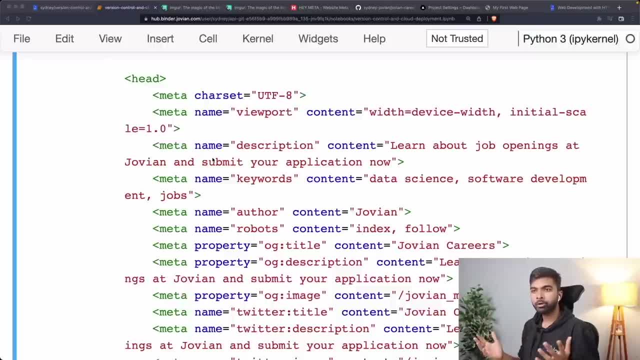 And we know how to do this. We just copy the code, put it into indexhtml, then stage the indexhtml file, then commit it, then push it. But before we do that, we're going to take this opportunity to maybe also 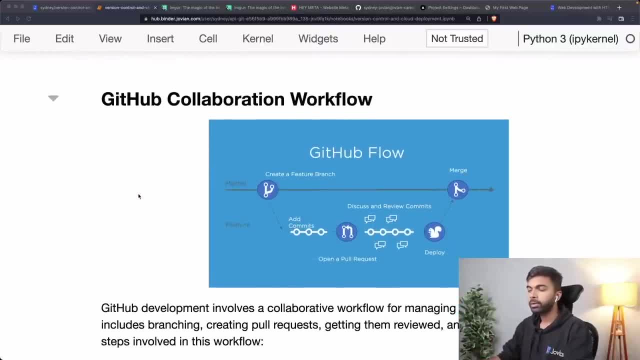 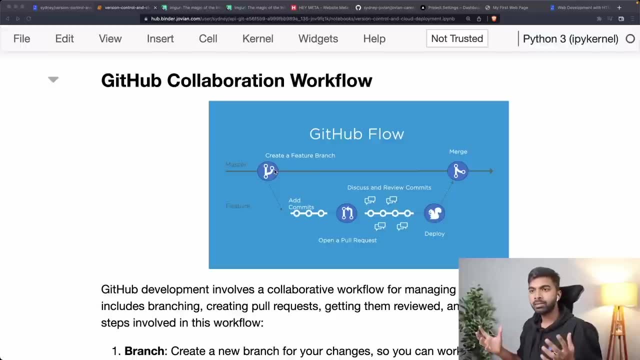 learn the GitHub collaboration workflow, because what is going to happen in the real world is that you you're not going to directly make changes to the main web. Okay, As you can imagine, let's say, Jovian, the website is running and before we actually make push any new changes, we may want to get them reviewed. We may also have a situation where multiple people are working on multiple changes and if they're all consists constantly pushing to the main branch, then they may all be just overwriting each other's code. 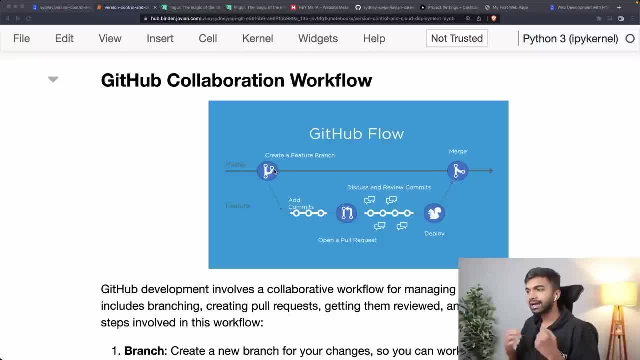 But that is why GitHub has this collaboration workflow powered by branches. So what you do is you have your main branch and then you have your main branch. Okay, So you have your main branch or your master branch. from your master branch, you create a feature branch, and we'll talk about branches in just a second. 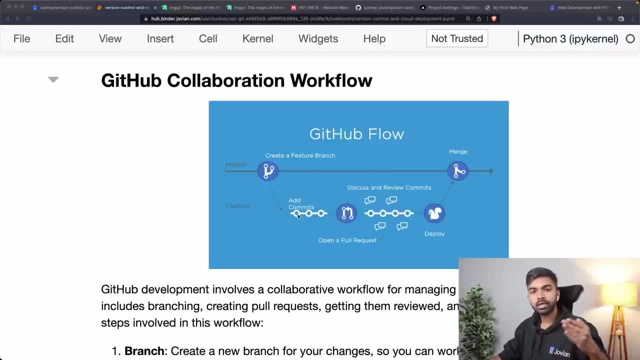 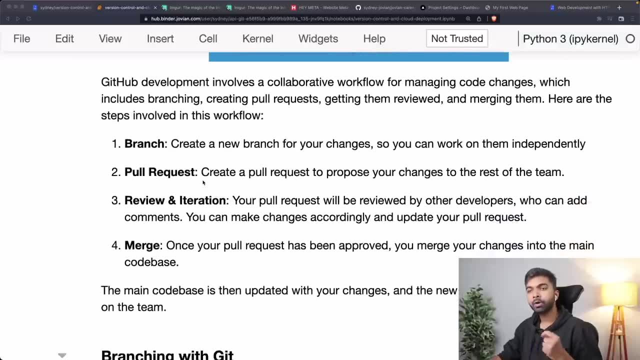 And then in that feature branch you add a bunch of comments. So, one by one, you keep adding comments into your feature branch. Then what you do is you create a pull request, So you using all the changes that you have put into your branch. 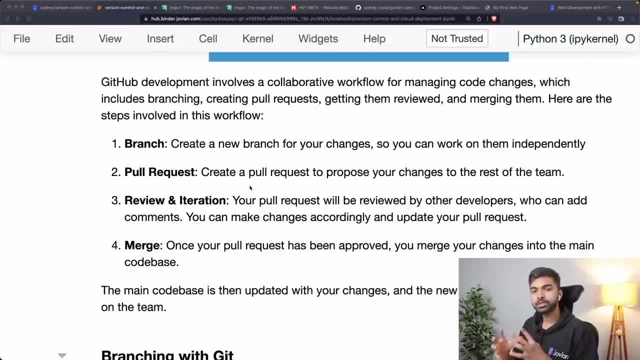 So far. you create a pull request on GitHub and in the pull request you can basically list out the changes you've made, the pull request. You also have all the code changes between your branch and the main branch and the team can then review your pull request. 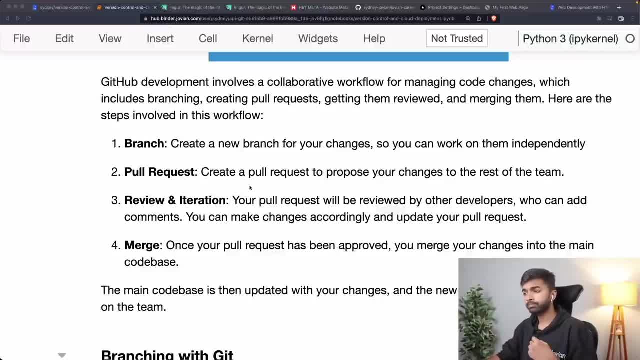 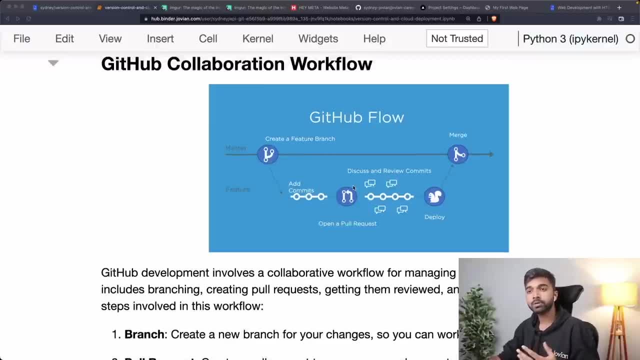 So somebody from the team can look at the changes you have made and they can make comments on your pull request. So they may make some comments and then you can then make more changes, make new comments based on those comments. You can fix the things that are not working as expected. 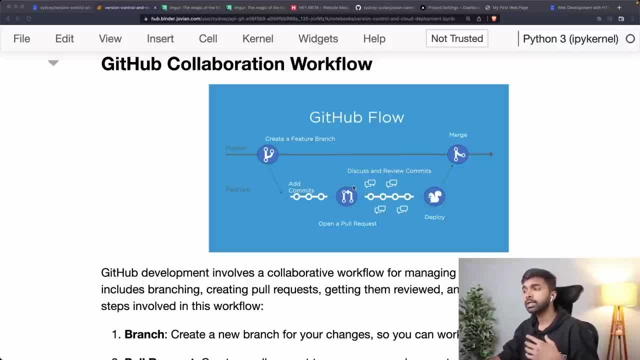 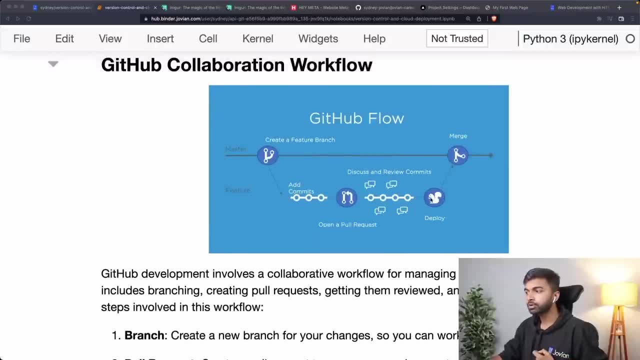 And once all the comments are resolved, somebody from your team can possibly approve your, approve your changes and once your changes are approved, you can then merge those changes into the main branch. Okay, so you can take the new changes and you can merge them into the main. 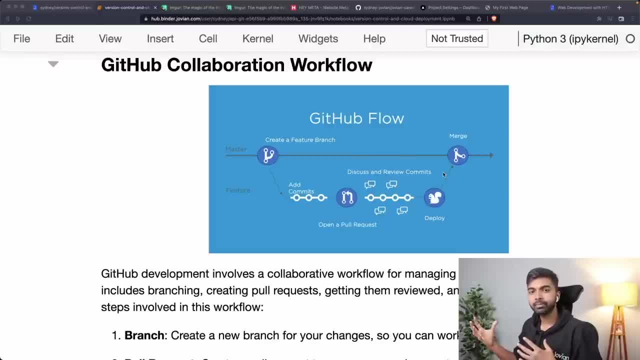 branch And then, of course, we have ourselves set up already. So as soon as the main branch gets changed after all this discussion and review, then it is going to get deployed automatically. So this is how we safely develop software: We take out a branch, which is basically we extract out a copy. conceptually, 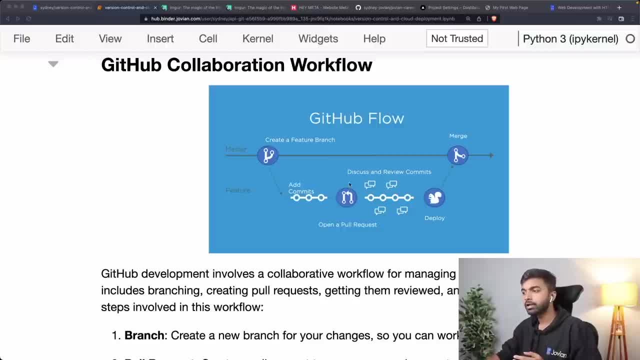 speaking, we make changes to that copy. We keep adding comments. We then set up a pull request. People comment on it, We make changes to it. We do whatever testing we need. We'll also see how to generate a copied version of our site, which is which: 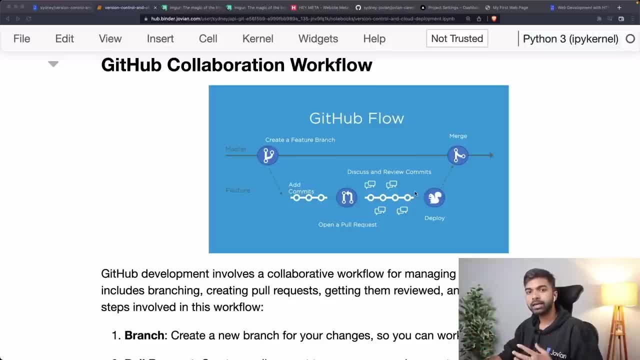 can be used for testing, And then, once we are ready, we approve the pull request, merge it back to master and that is going to trigger a deployment. So that is how the GitHub collaboration workflow works, And it's not just that you will be using a single branch at a time. 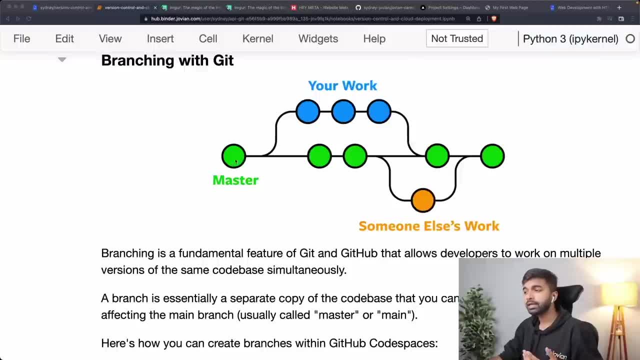 But here's what might happen: that you may have your main branch somewhere and then somebody. you may start a new branch. You may start making some changes and then some changes may get added to the main branch from other people and then somebody else may start another branch. 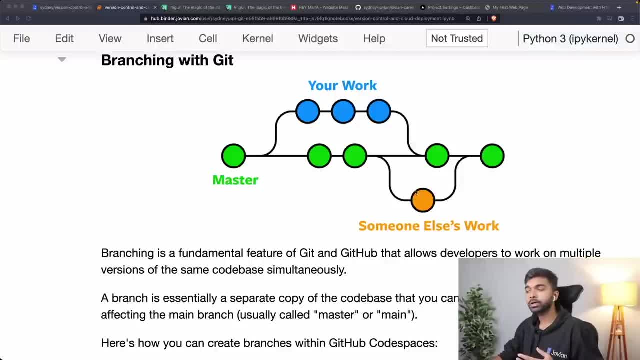 and then your branch may get merged and then their branch may have to get merged. So this is how the GitHub development workflow works. Anytime you want to build a new feature, you create a new branch, make changes on the branch, get that reviewed, get that approved, merge it back into the 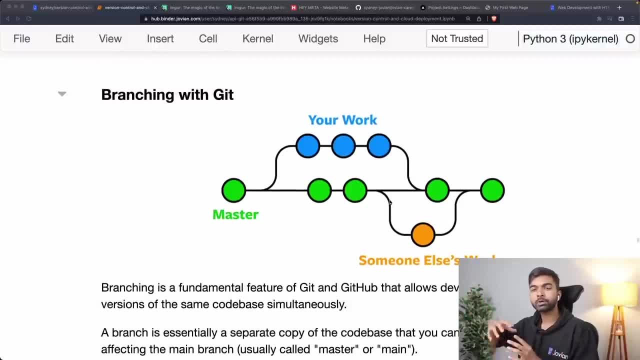 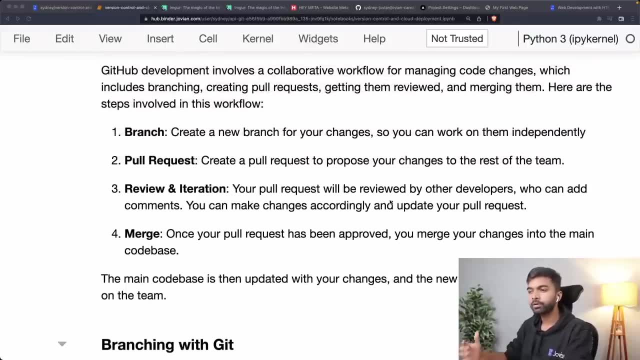 main branch, And the main branch is the source of truth for what is going to go live on Vercel or whichever deployment platform you use. So this is the workflow that we're going to follow, And the first step in this workflow is to create a branch. 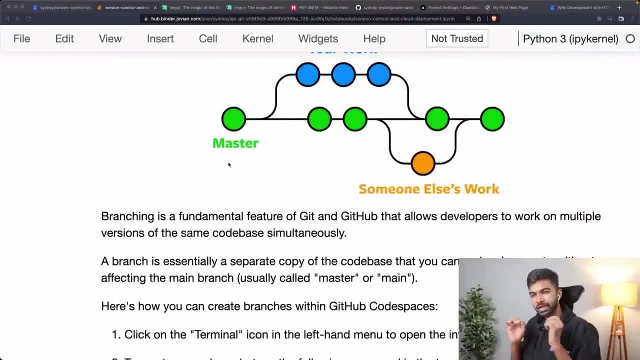 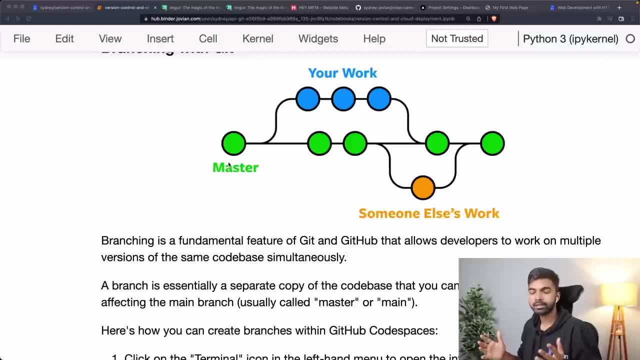 So what is a branch? Well, a branch branching is a very fundamental feature of Git and GitHub that allows developers to work on multiple versions of the same codebase simultaneously. So you can use it to work on five tasks at a time, or five features at a time or five. 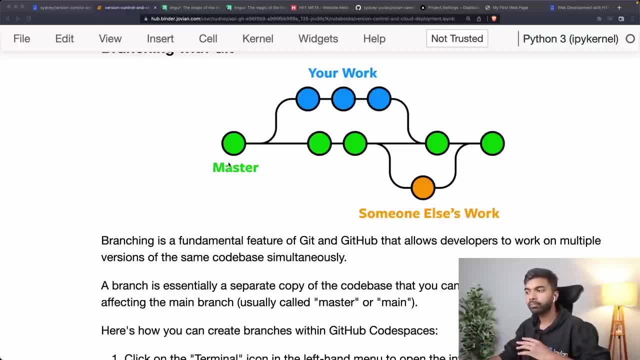 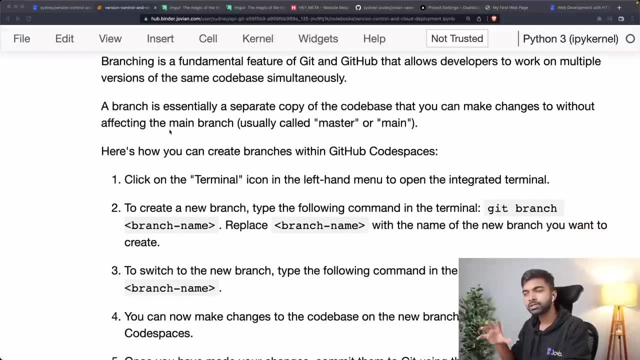 different people can use it to work on different features without disturbing each other's code. Okay, And a branch is essentially a separate copy of the codebase, conceptually speaking, that you can make changes to without affecting the main branch, which is usually called main. 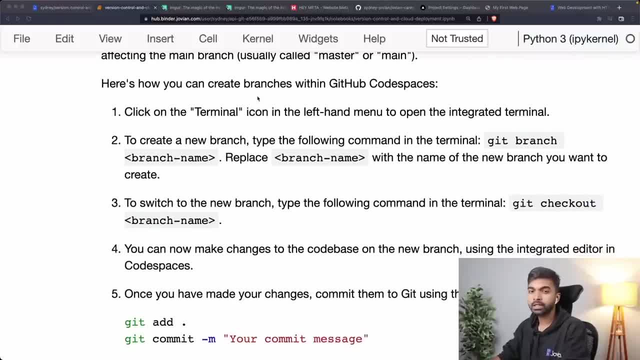 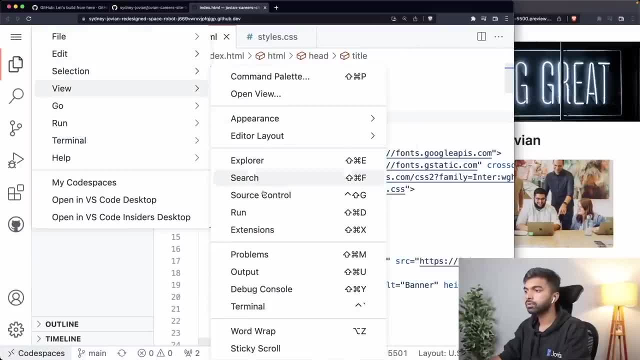 or master. So here is how you create branches within Git or using Git or within GitHub code spaces. First we open the terminal. So once again I go in here I say view terminal. Now I have the terminal open here and let me close the sidebar. 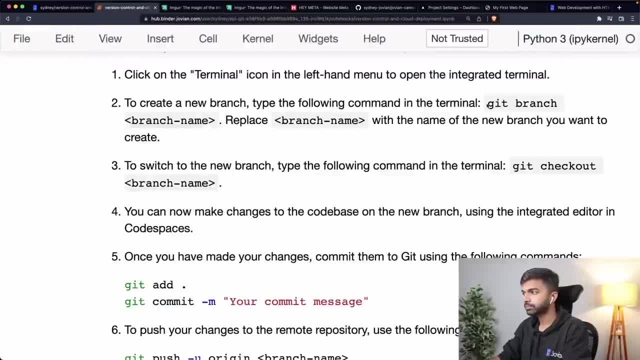 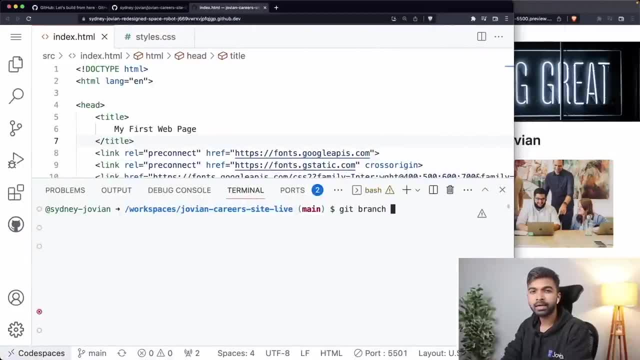 So the first thing you do is you type git branch And then you type git branch And then you type a type, the name of a branch. Okay, so you'd say git branch And I just want to add meta tags here, So I'm just going to call this branch, add hyphen, meta hyphen tags. 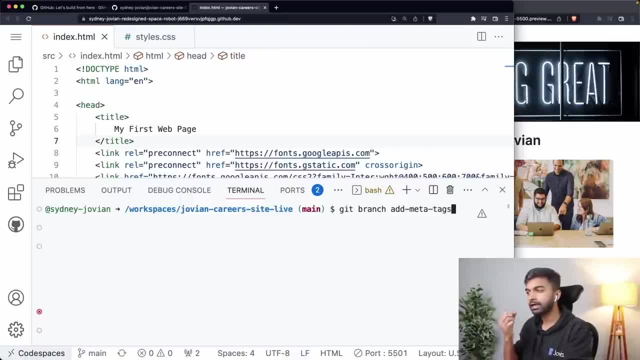 So you always use lowercase letters like add hyphen, meta hyphen tags, all lowercase, and you always generally separate by hyphens. You can also separate by underscores if you want. One other convention is to also maybe put your username before the branch. 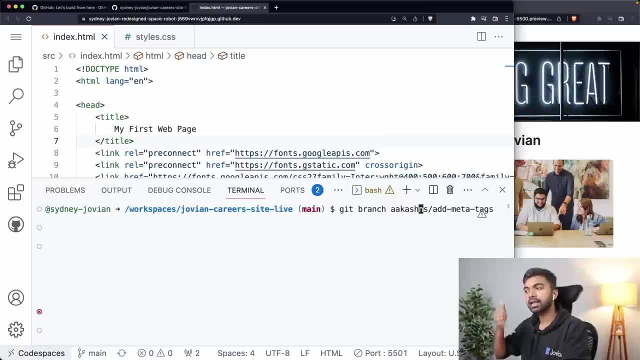 So you could, I could also create the branch as such. Akashin is slash. add meta tags. But this is a good convention so that multiple people don't end up creating branches with the same name accidentally. In my case, I'm going to- I'm going to just use the shorthand a for myself. 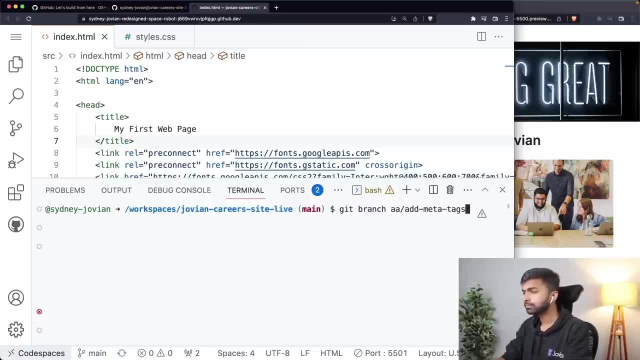 So a slash add meta tags. That's what I use at Jovian. Okay, so we are creating a branch called a slash add meta tags. Okay, the slash does not have any special meaning. It is simply a separator that I'm using. 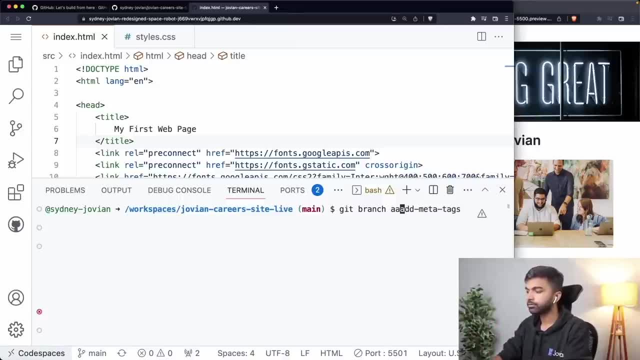 I could also have said: a hyphen, add meta tags, and it would be the same thing, But it's just a little nicer to look at. Okay, So a hyphen: add meta tags. So now I'm creating a branch. So a branch has been created. 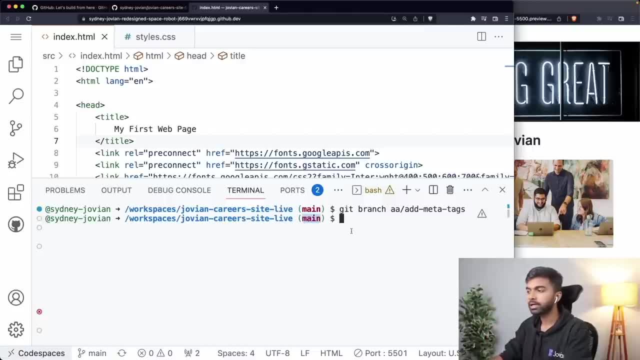 But we are still on the main branch here. You can see, here I'm still on the main branch. So now we need to switch to this new branch that has been created. Now the way to switch to a new branch is using the git checkout. 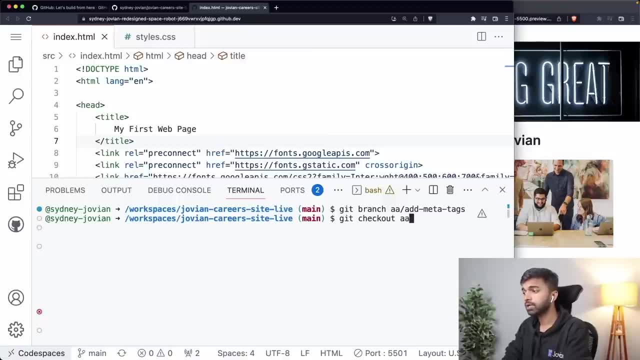 So you say git checkout and then you type the branch name. So a slash- add meta tags. Now we have switched to the branch. a hyphen add, a slash, add meta tags. Great, And that is something that is displayed here as well. Now that we have switched to the branch, we can now start making commits into this branch. 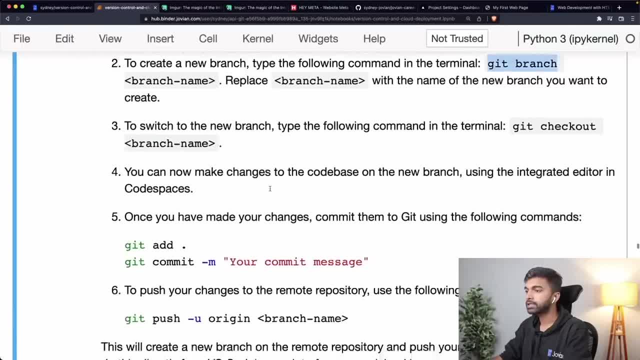 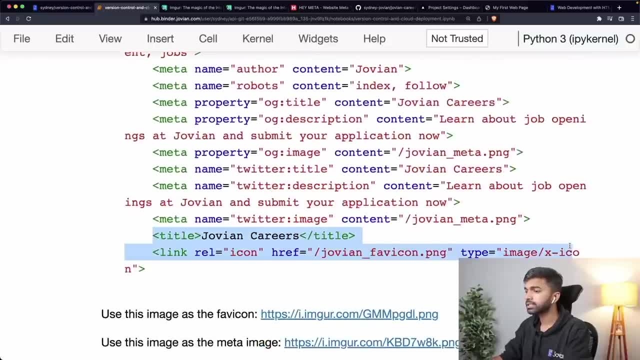 So here is how I might go about making some comments. So I might first- let's see here. I might first maybe just replace the title and the favicon. So let me just grab the title and the favicon here And I'm just going to replace that over here. 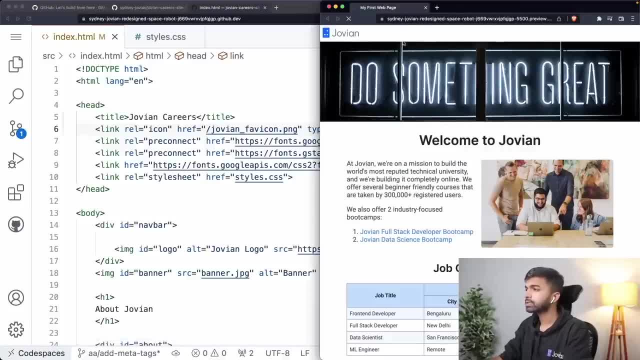 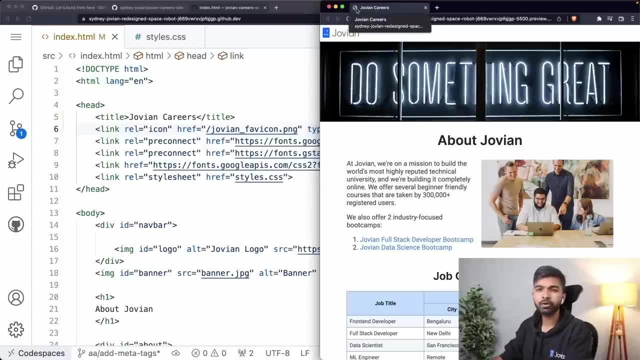 Okay, And I will just test that. So now when I reload the page, You can see that now we have Jovian careers And, okay, this still doesn't have the favicon. Maybe the favicon will come in when we actually deploy. 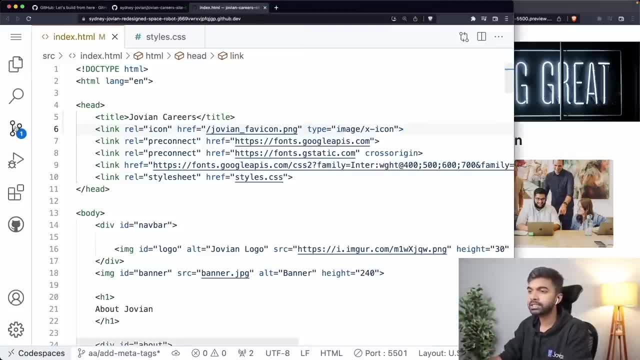 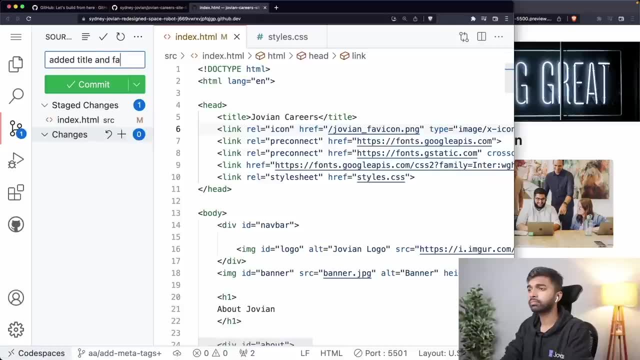 But looks like at least the title has changed. Okay, so I've made one significant change. So I'm just going to stage this change, I'm going to say added title and favicon And I'm going to commit. Okay, I'm not going to push my branch here. 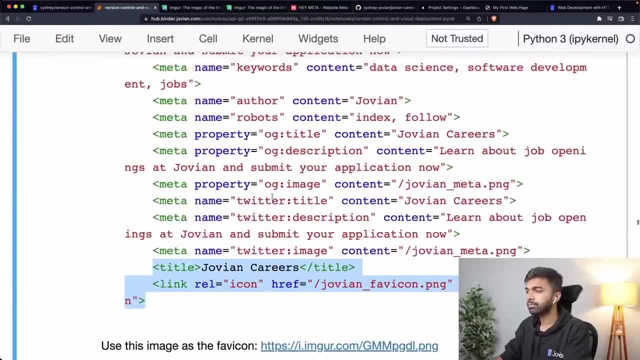 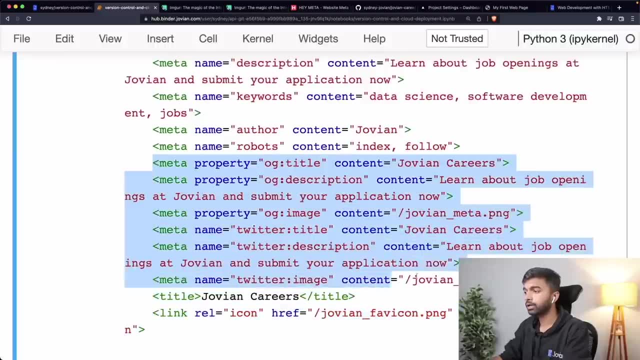 I want to make a few more comments before I push my branch. Okay, then maybe I might figure out. Okay, I might talk to the marketing team. I might figure out what they want as the OG and the Twitter meta properties. So I will add those. 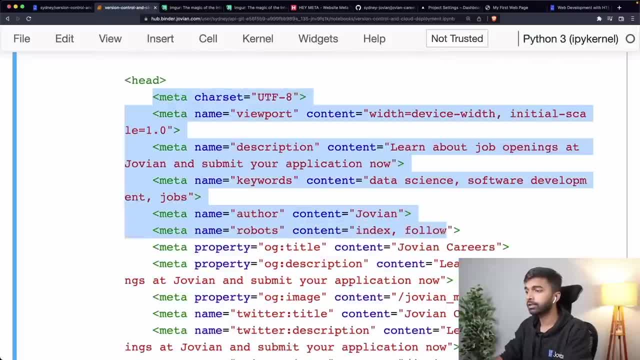 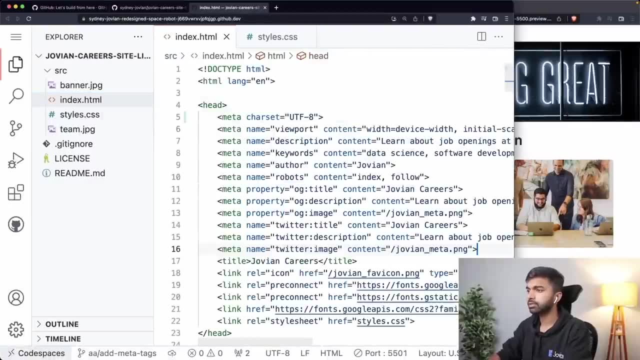 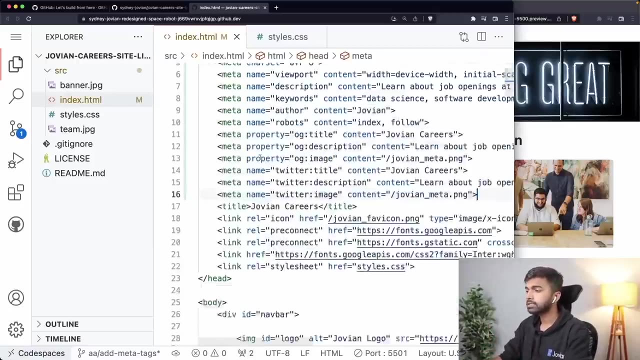 And then I might talk to maybe the engineering team and figure out that, Okay, what are the other meta properties I require? Let me grab all of the remaining meta tags and let me come in And let me just paste them here. Okay, so I'm just simulating an example where you will be making small changes step by step and making multiple commits. 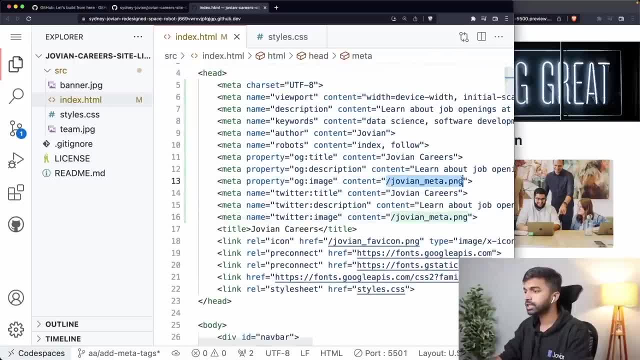 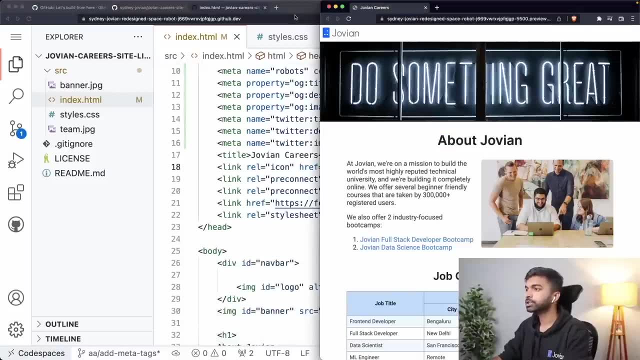 So I've gone ahead and made these And, of course, now for this OG image and for this Twitter image, I need to actually upload this image file, And I also need to upload this favicon file. Okay, that's why the favicon is not showing. 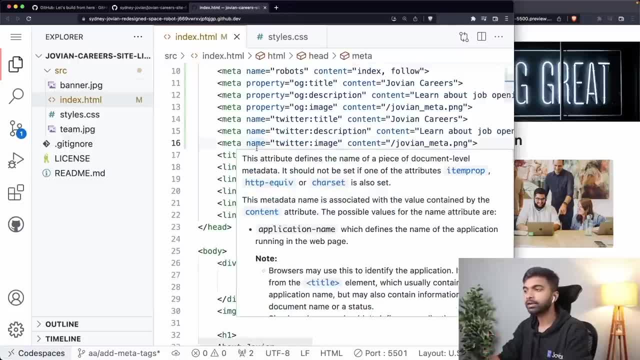 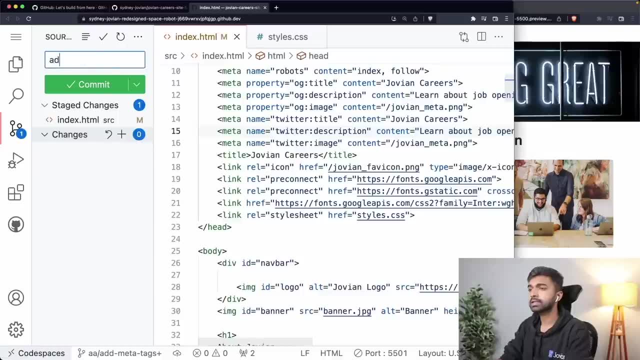 So I'm going to let me first add the meta tags. I'll create another commit where I upload the files. So again I can go in here I can say add the changes I can commit, Let's say added meta tags. 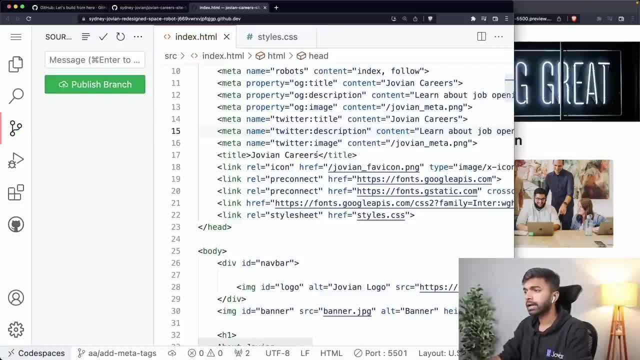 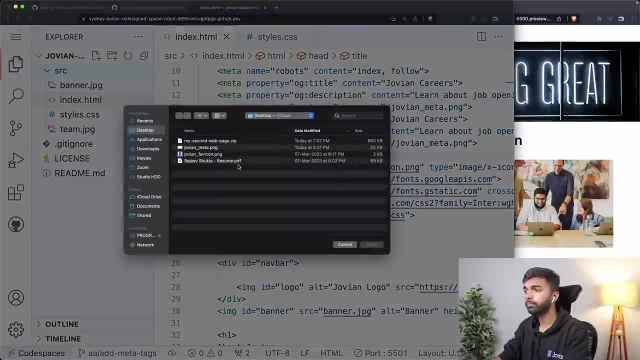 I can commit, Great, perfect. And now I can go ahead and I can actually upload the files. So let's say, I can commit, I can actually upload the files, so I can come back here. I can say: right click, upload. Let me grab jovianmetapng, jovianfaviconpng, upload them. 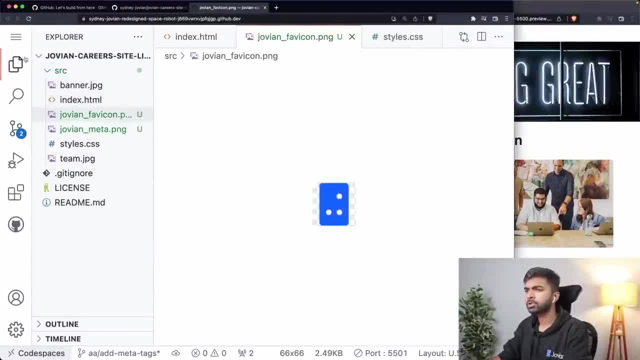 They are added as well, And once again I can go in and I can also do this from the command line. So I say view terminal and I say reset And let me just do git status. Okay, looks like there are a couple of new files. 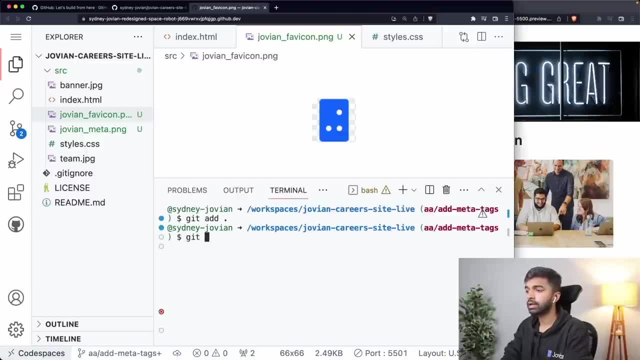 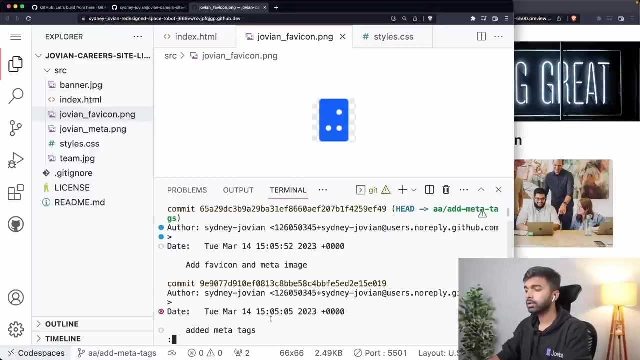 So let me do git add And let me do git commit minus m add favicon and meta image. Okay, All right, So I've not pushed my changes yet, So I have a bunch of commits here on this particular branch If I just check git log- or I can actually just if I just want to see the list of changes. 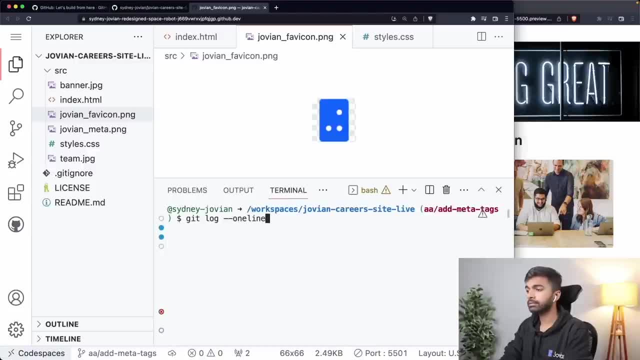 I can say: git log minus minus one line. Okay, So I've. so my branch AA hyphen. add meta tags is at the commit. add favicon and meta image. Before that I have another commit. Before that I have another commit. I've made a bunch of commits. 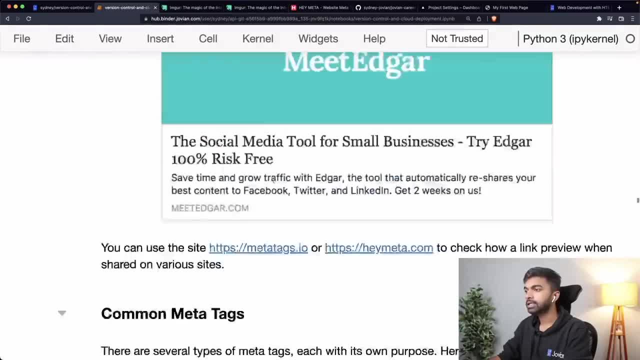 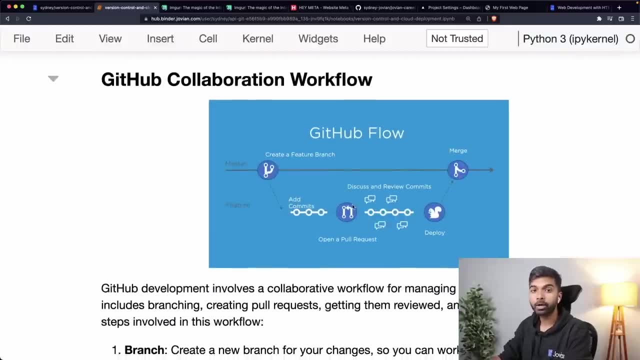 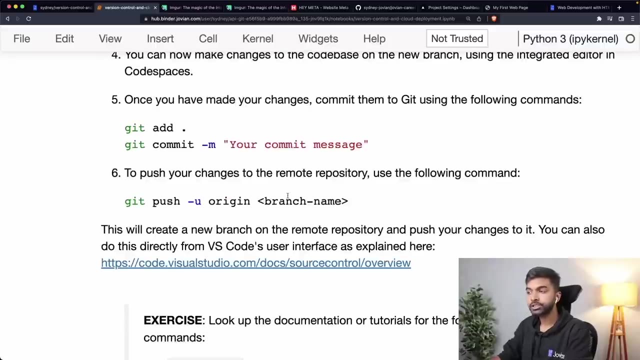 Now, once I have made a bunch of commits, once I have made a bunch of commits, I can then open a pull request. So to open a pull request, here's what I need to do. First, I need to push my branch or my changes to the remote repository. 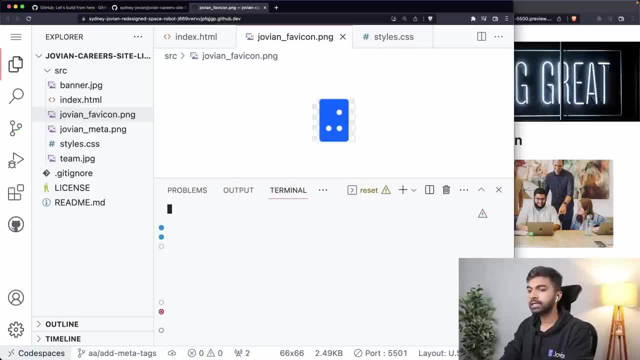 And the way I can push them is by saying git, push origin, followed by branch name, AA, hyphen, add meta tags. Okay, Of course I can also achieve the same thing by just clicking publish branch here, But I'm just going to do it from here. 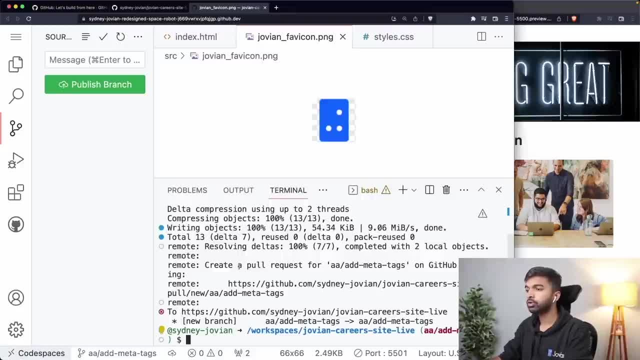 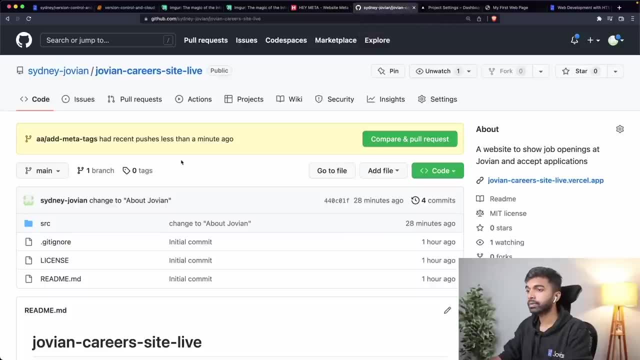 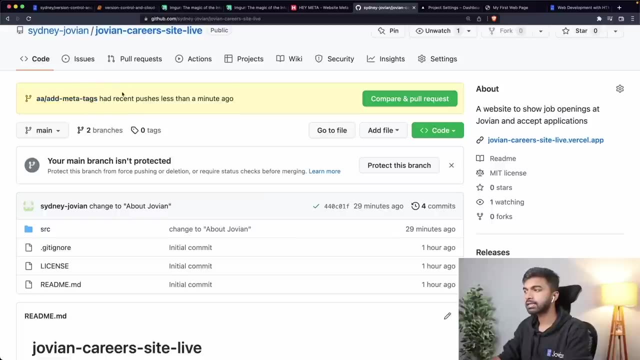 And once that is done, you can now see that a new branch will have been pushed to the GitHub repository. How do we verify that? Well, if I open the GitHub repository and I just reload the page, you can see this. there's this message here that this tag, this, had recent pushes. of course there's this. 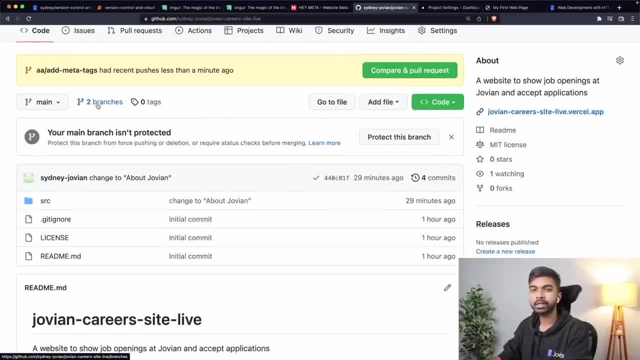 trigger. But you can also see here that we have two branches now. So earlier this was just saying one branch. I can actually go and select the other branch. So the commits that I've made together, I can package them as a branch and I've pushed. 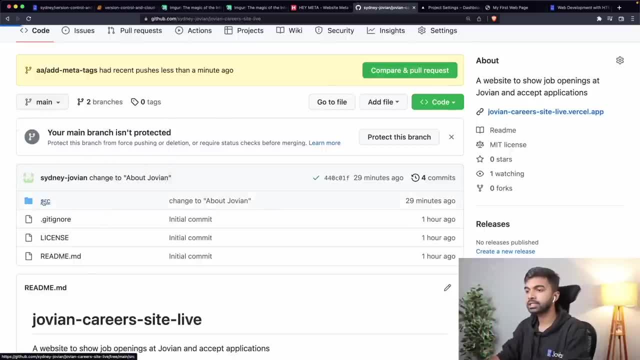 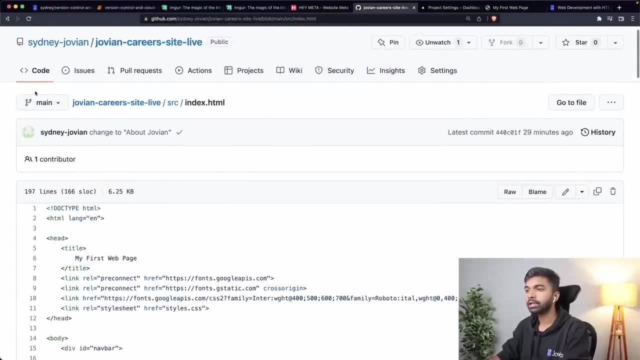 it to GitHub. And now I have this on the main branch. you can see here that SRC index dot HTML Doesn't have any of the meta tags. my main branch is unaffected, But if I change to the branch, add meta tags. 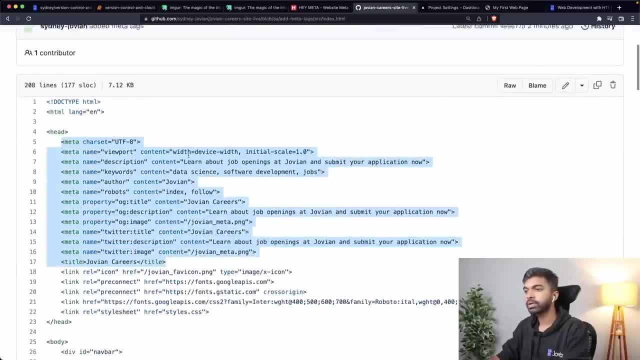 On this branch. you can see that all the tags are present. Okay, So this is how you push branches. Now what you can do is you can make more commits, you can push the branch again. So you decide what you want to do. 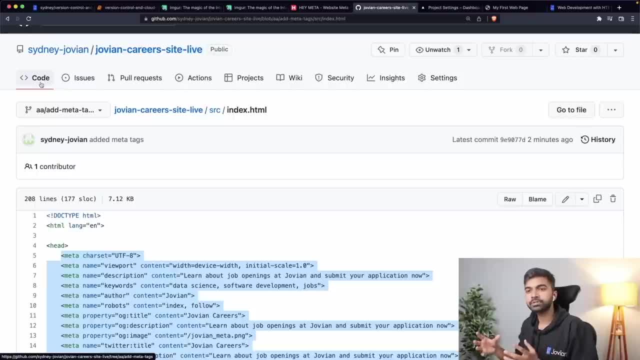 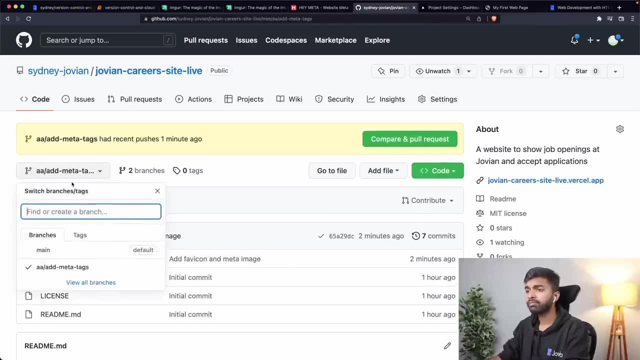 Typically, any small change I make, I make a commit And then, once I have a bunch of small changes that are significant enough, I push the branch. Okay, But coming right back, Now we have pushed, let me come back to the main branch here. 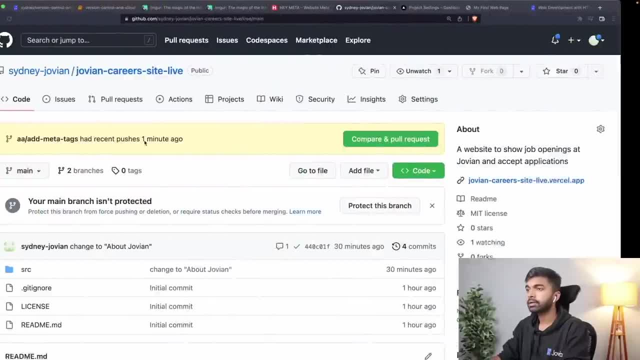 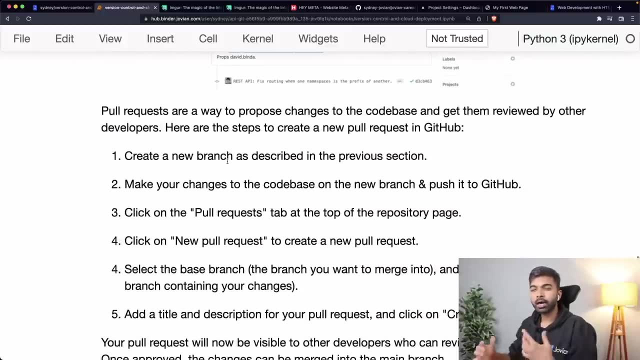 Now that we have pushed the branch, the next step is to create a pull request. So how do we create a pull request and what are pull requests? So pull requests are a way to propose changes to the code base and get them reviewed by other developers and then get them merged back into the main branch. 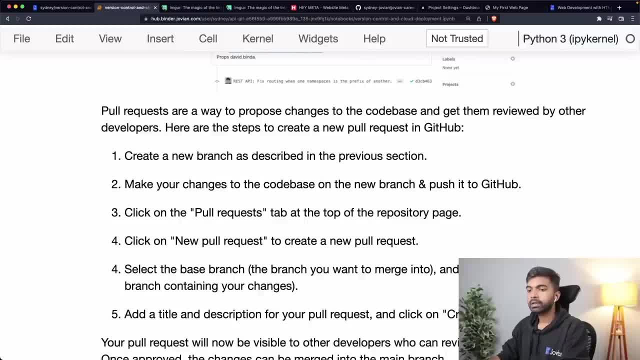 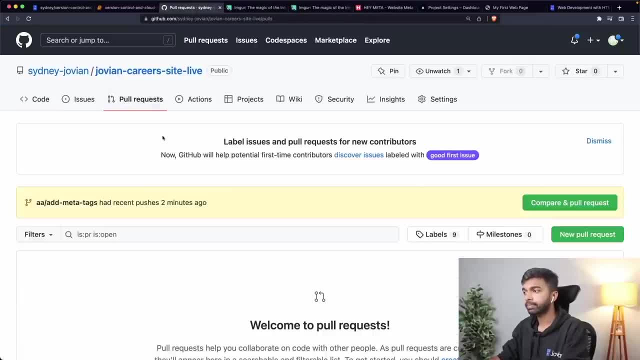 All right, So let's create a pull request. So first we are going to come back, We are going to go into the pull requests tab and into the pull request tab Again. you can see that there is notification- here GitHub tries to be helpful- where it tells you that if you recently pushed a branch, 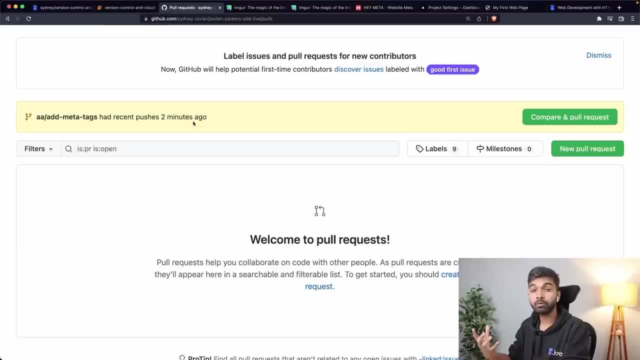 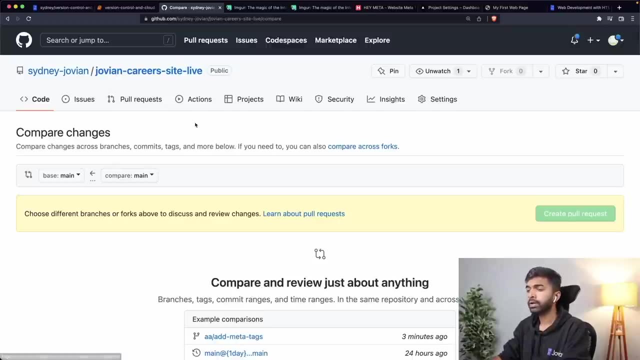 it'll tell you. it'll ask you if you want to create a pull request. But in case this notification is not showing up, you can click new pull request. Okay, And now you can select the base branch, which is where you want your changes to eventually. 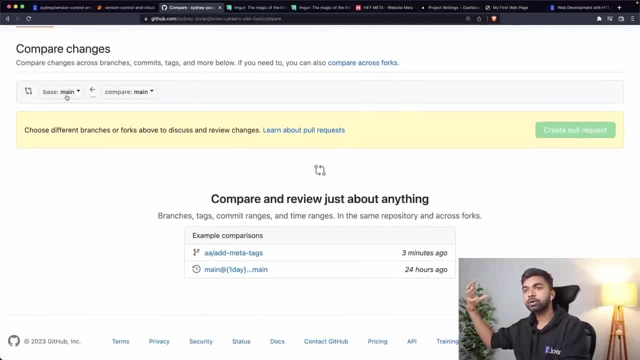 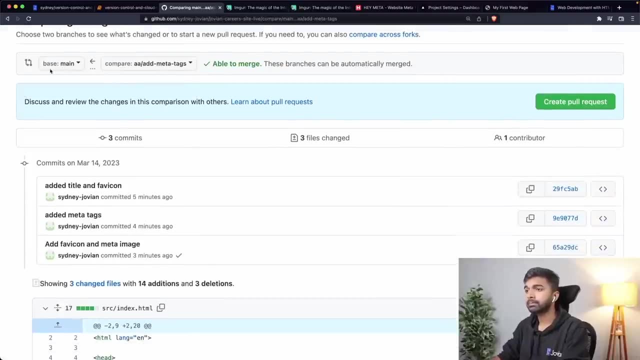 go and the branch where you are making your changes, which is add meta tags. Okay, So now you can see that you can create a pull request. Okay, So now I've selected that these are the two branches and I can actually verify what are. 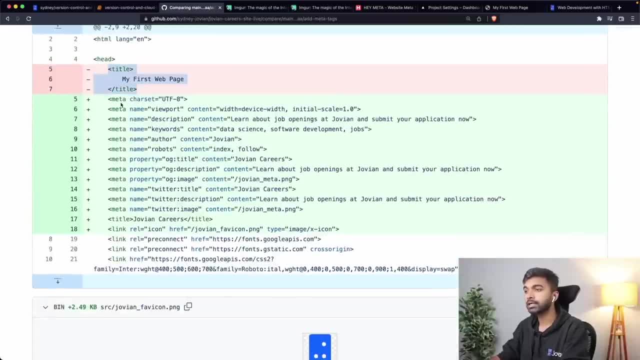 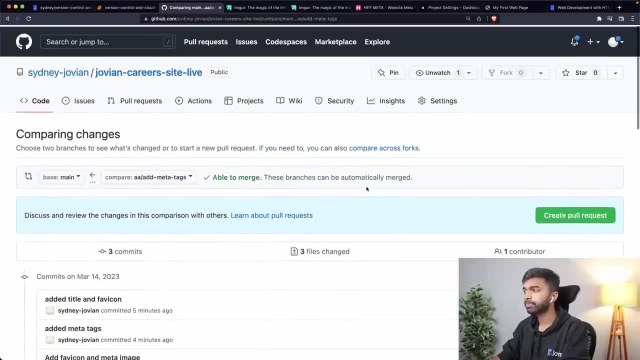 the changes. So it seems like from the main branch I want to remove this existing title and I want to add a bunch of these meta tags and seems like I also want to add a couple of images files. Okay, So I can review the commits that have been made on this branch. 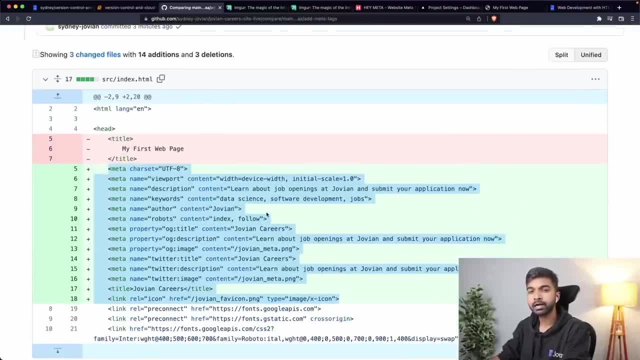 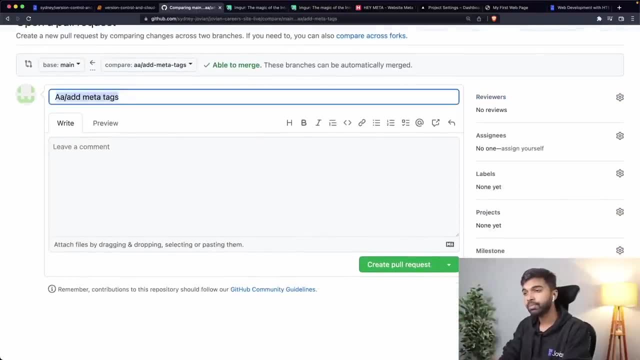 I can review the changes between the main branch and this new branch that I'm proposing, And then I can click create pull request And here I can give the pull request a name And typically you want to give this a description of the change. 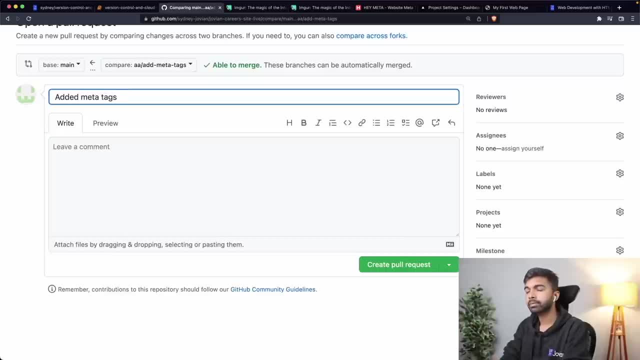 So added meta tags, title and favicon, And it's also a good idea to maybe provide more detailed description of the changes So you can say: changes One is added or updated the title tag. Then you can also mention: Okay, Added images or favicon and meta poster or meta banner. 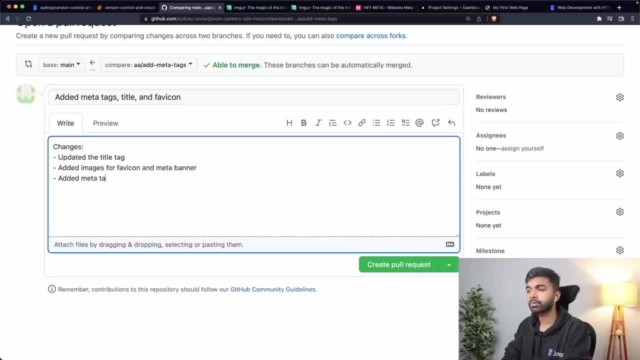 Then you can say: added meta tags, including OG and Twitter tags. And finally, you can also mention: added the favicon link tag. Okay, Now let's say you've tested these changes. You might also want to say what you've tested. So test cases, checked. 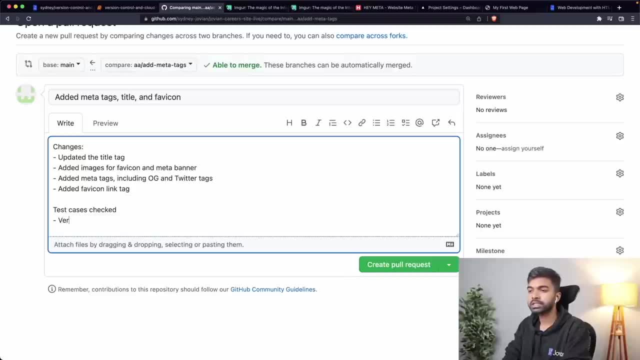 Okay, So you can say something like: verified the title showing up And maybe you might want to verify later and add later that you verified the favicon showing up and you verified the meta tag showing up, Okay, And then you click create pull request. 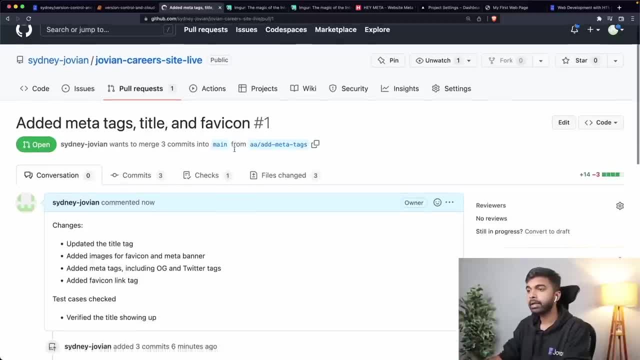 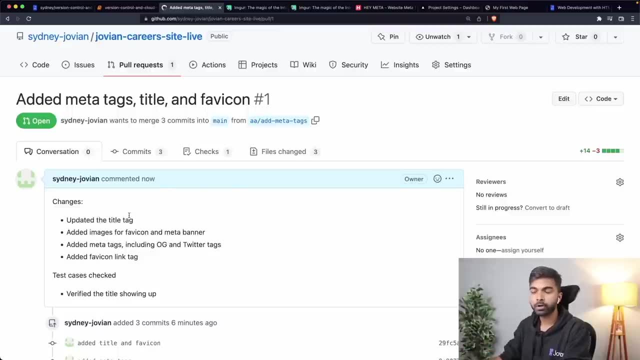 So that's great. Now the pull request is created And now somebody else on your team who is a collaborator on this repository can go ahead and review this pull request. So let me first go ahead and add a collaborator here. So I'm going to go into settings. 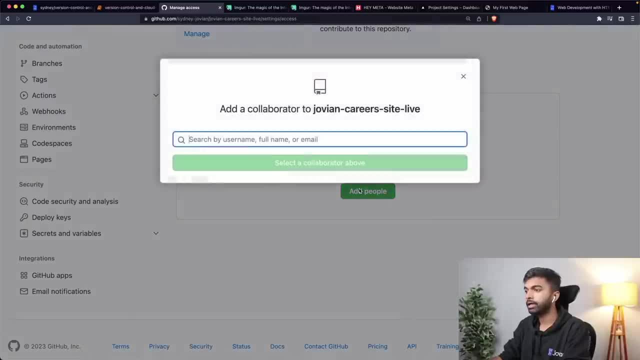 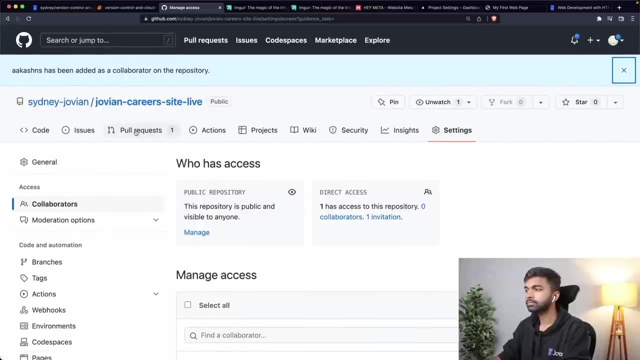 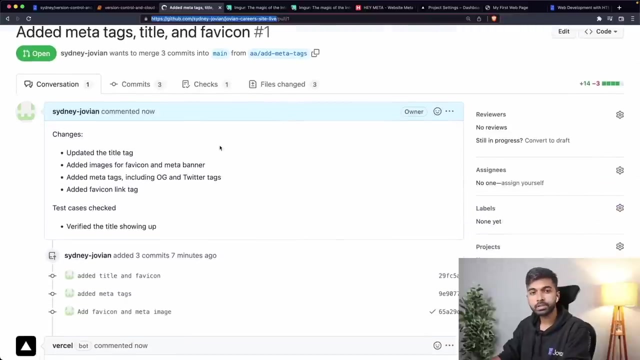 I'm going to go into collaborators And I'm going to add a collaborator here. Let me just add Akash NS, And I'm going to invite this collaborator. Let me go back to the pull request. Okay, So this, this pull request now has a description and there is this: files changed, which contains: 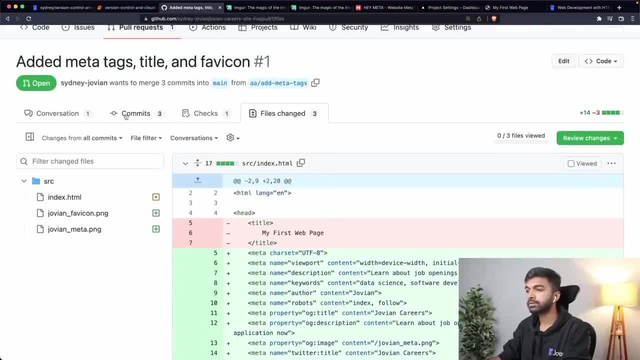 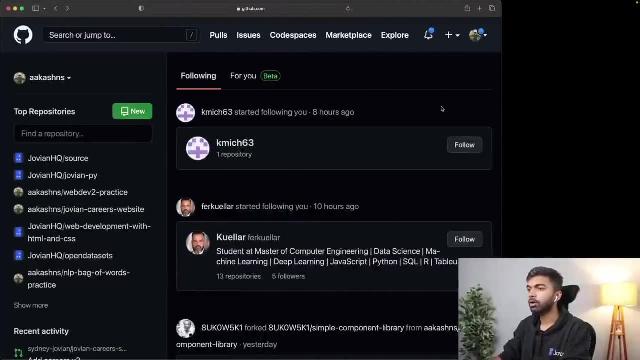 information about the files that have been changed, So people can review that as well. It also contains information about the commits that have been made. So now let me go in and log in from a different account. So I have a different account logged in here and I'm just going to accept the invite first. 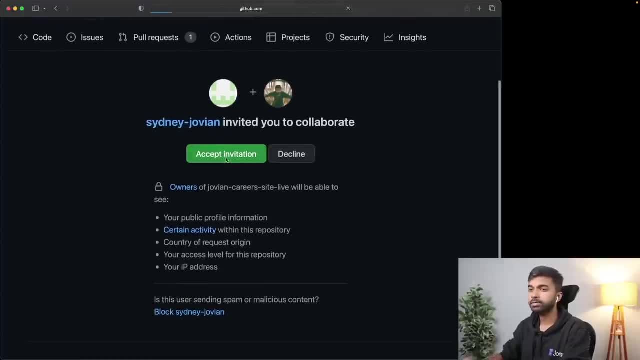 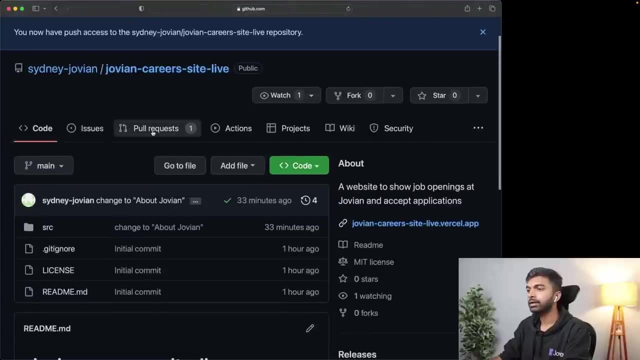 I've been invited as a collaborator here So I'm going to accept the invite. So anytime somebody you invite somebody as a collaborator, they get sent an email and they can accept the invite. Okay, Now that I've accepted the invite, I can go here into the pull requests tab. 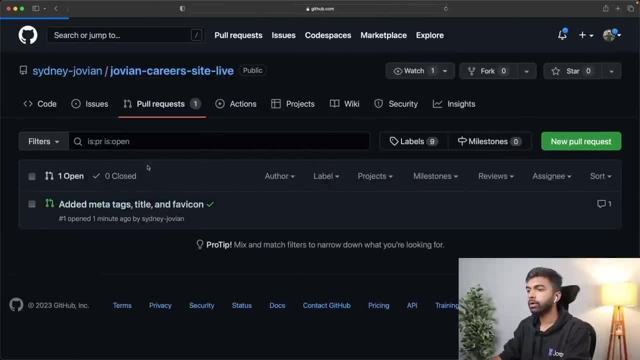 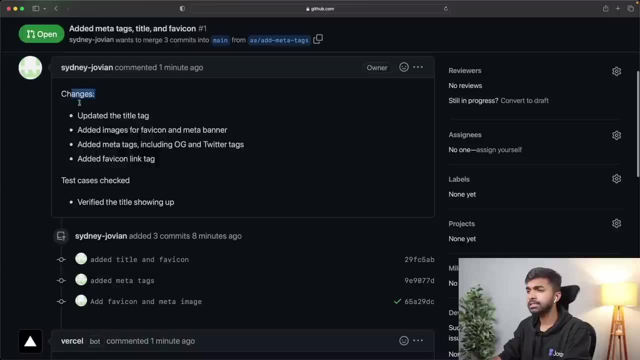 And I can go check the pull request. You can. I can see that. Okay, Sydney Jovian has invited me or has created this pull request. I can check. Okay, These are the changes that have been made. I can maybe go in, and then I can go in and maybe leave a comment. 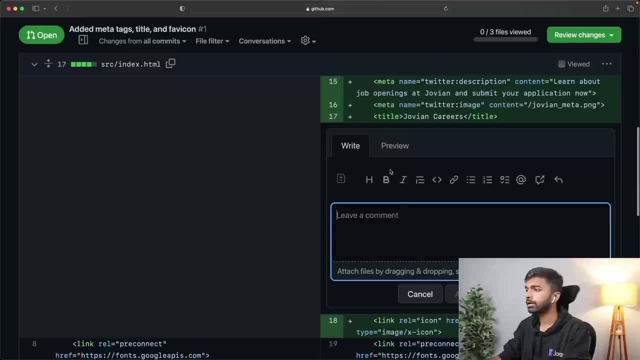 So let me say, for example, I don't like this title, I want it to be a little longer. So I can say: make the title longer please. Maybe at least 24 characters, Okay, And then I can just start a review. 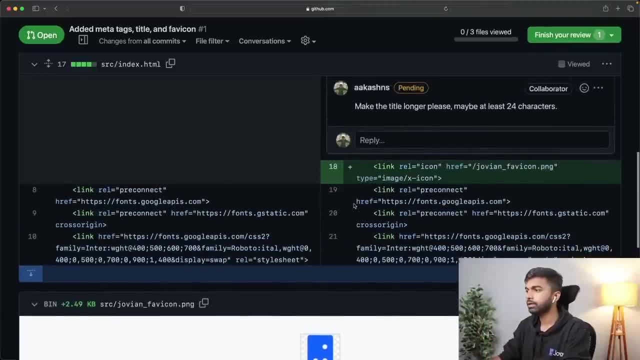 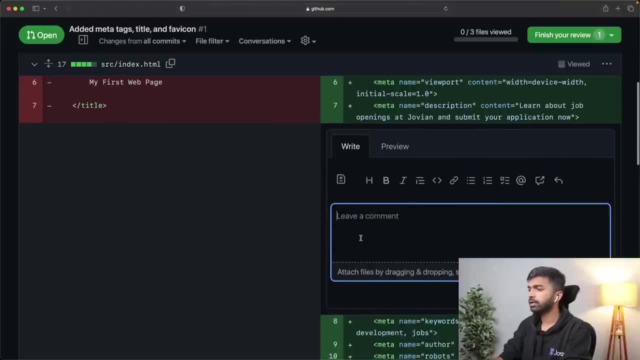 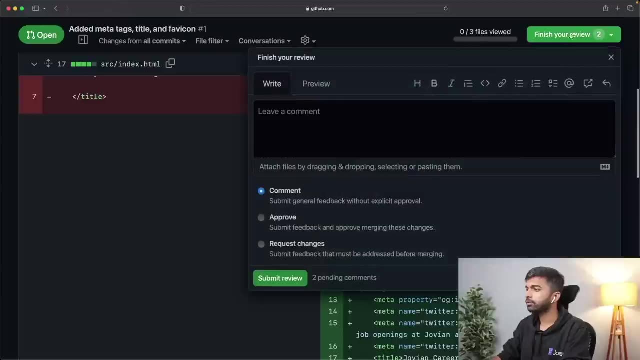 And I can add a bunch of these comments. So I can add a comment maybe about the meta tag, meta title here as well somewhere, Let's see, This can be improved a bit, And so on. And once I'm done with reviewing I can just say I can request some changes or I can approve. 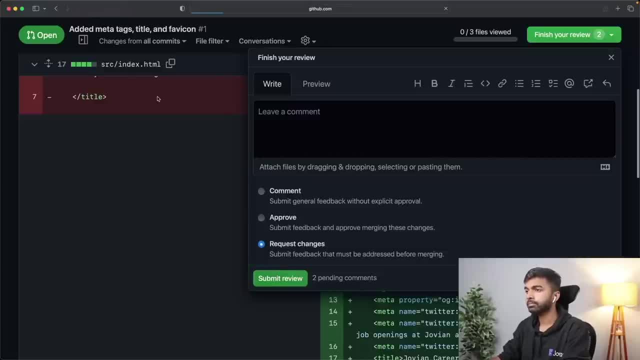 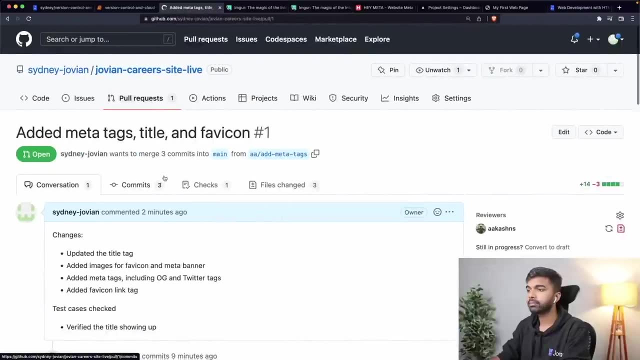 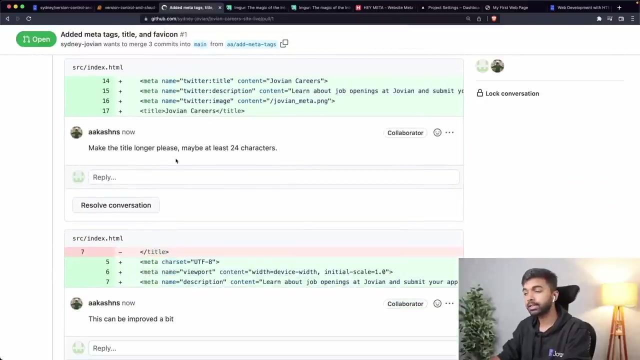 and I can click submit review. And once I've clicked submit review, then these changes have been pushed back And now Sydney Jovian can once again go through the changes, go through the comments that are made and make those changes. Okay. 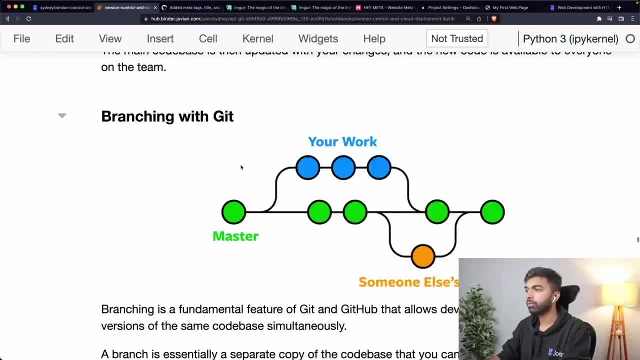 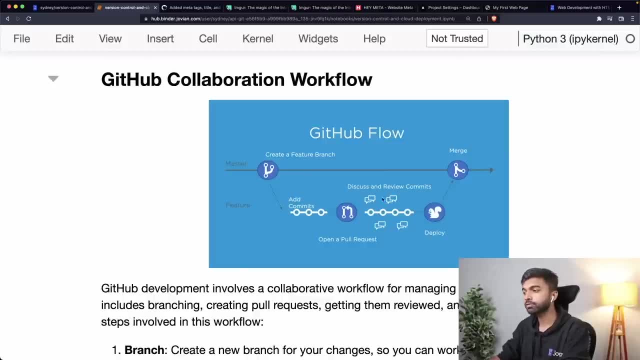 So, so again, we are just trying to implement this workflow here, where you create a pull request and then somebody posts a bunch of comments and then you create new comments to fix those comments and you keep repeating this process till they're happy with it. 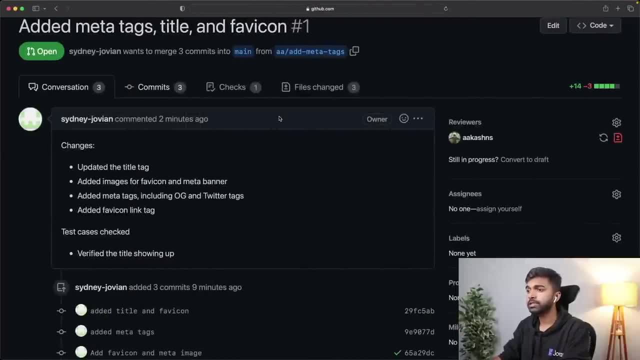 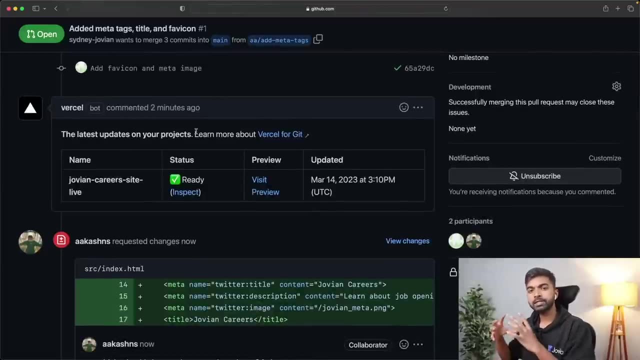 Okay. So one other thing I want to show in this process is that if you see there is a Vercel bot that has added a comment here, What Vercel has done is, whenever Vercel notices a pull request in your GitHub repository. 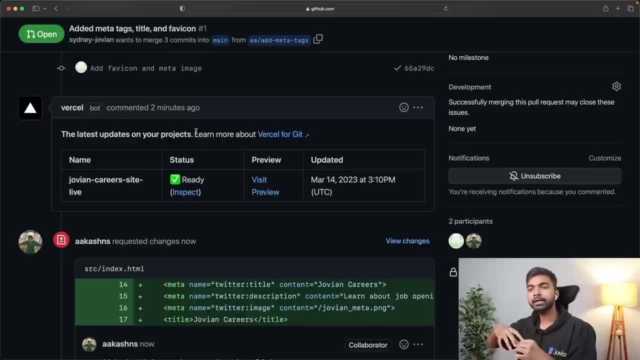 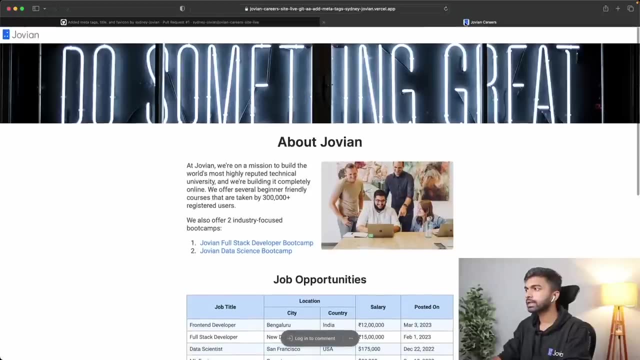 it takes the code within that pull request and it automatically creates a preview deployment So I can click this visit preview and I can actually preview the changes. Okay, I can see here that now it says Jovian careers instead of my first webpage. 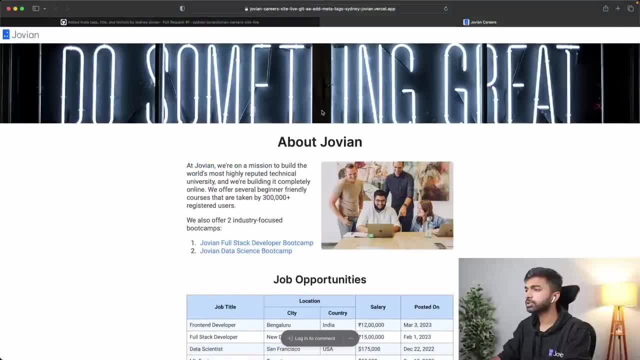 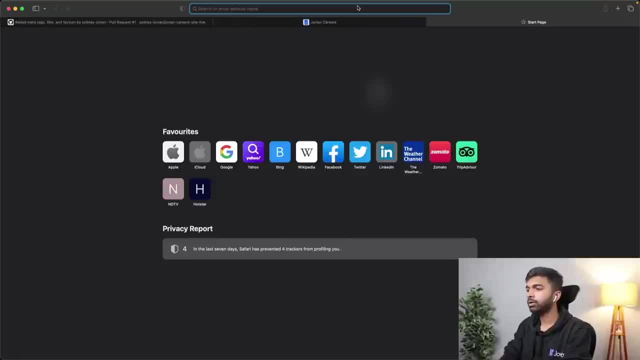 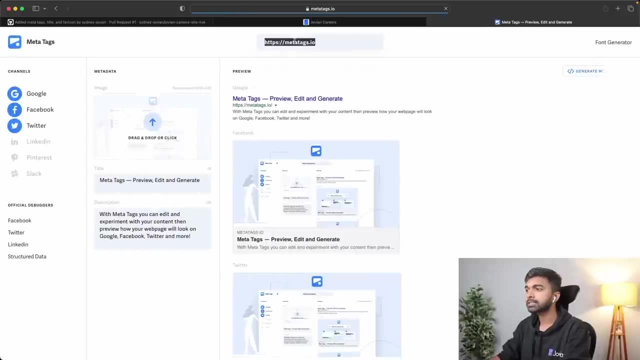 And there seems to be a bunch of this image seems to be showing here as well And there are no changes in the actual page. but if I were to maybe take this and maybe go into metatagsio, a platform for checking meta tags, I can actually check that. 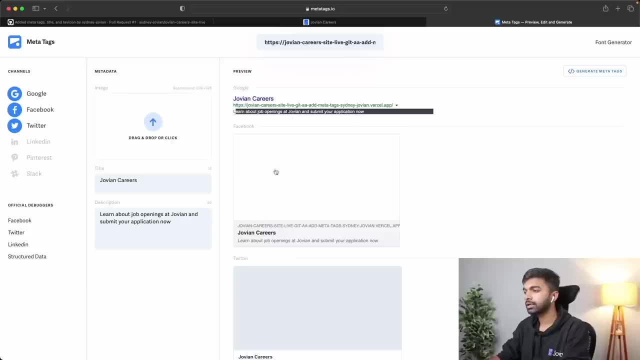 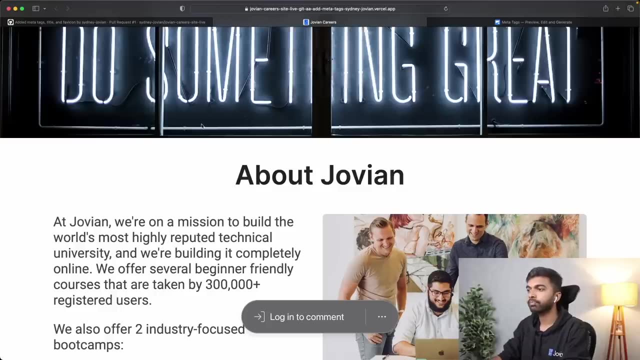 Okay, It is showing Jovian careers and it is showing a description here. Image is not showing up. I can investigate why the image is not showing up, but it looks like the meta tags are now showing up. Okay, So one of the nice things about using Vercel: what it takes, it takes your branch, your 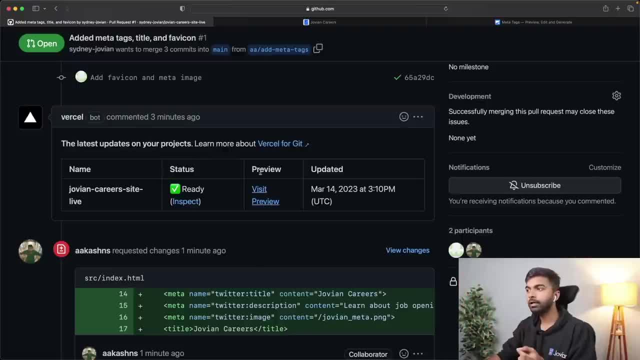 pull request branch. it deploys that and it adds a link to that without disturbing your original page. So you can see Jovian careers site. This is like that branch preview but your original site, which is over here, Jovian- 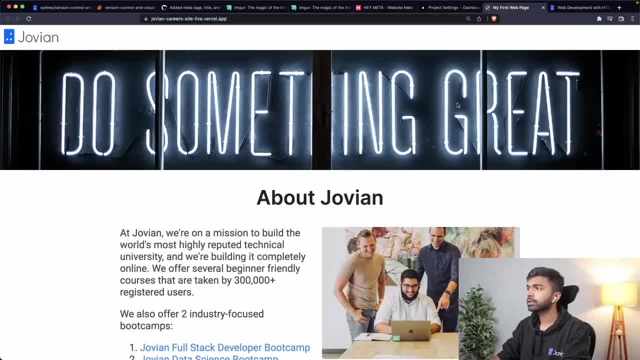 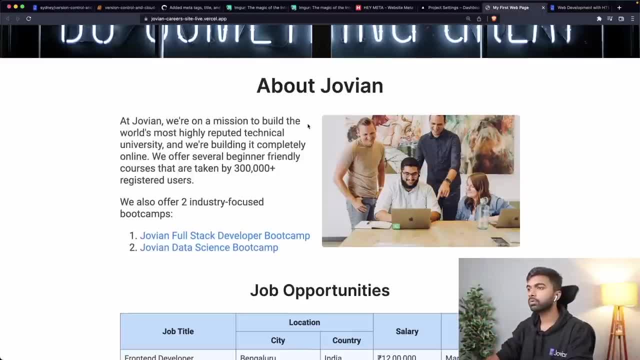 careers site still says my first webpage. it is not updated. So your main branch is saved. but for your pull request, you have a preview or deployment that you can study. Okay, All right, So let's go in and fix these quickly. 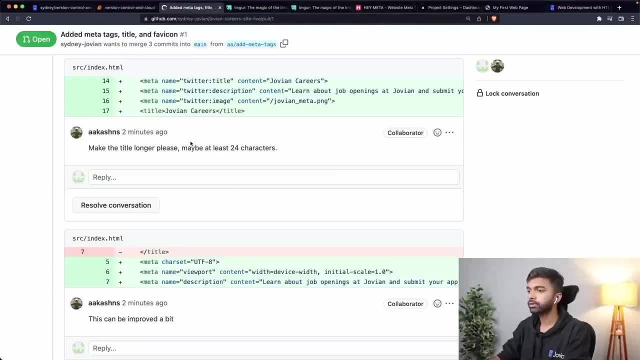 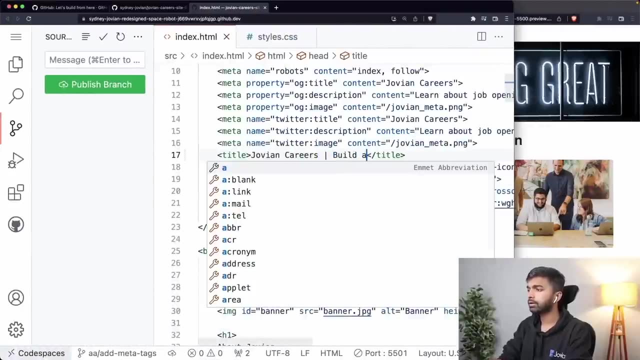 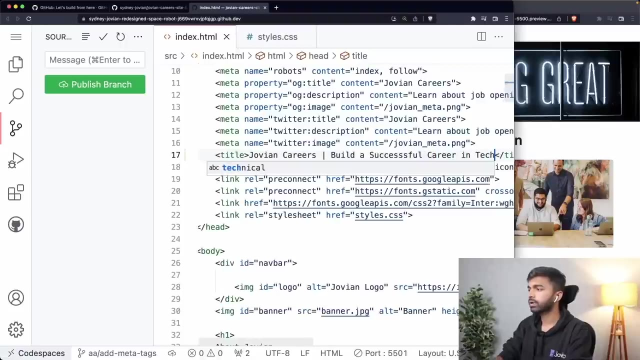 So I'm just going to go in and fix these comments. So there is a comment here that says: make the title longer please, Maybe at least 24 characters. I'm just going to add maybe here: build a successful career in tech. 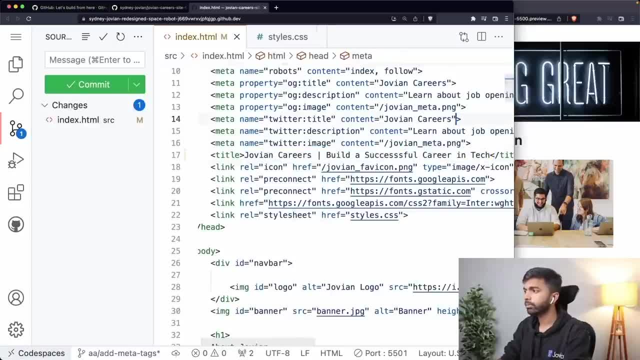 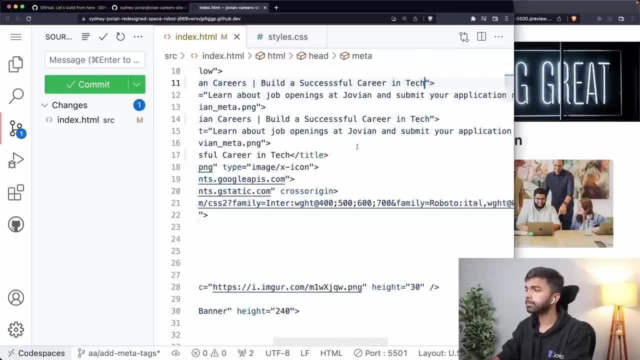 I'm going to add the same title here back in the OG title, like that. Okay, I've made. I fixed the title: learn more about job openings and submit your application now. Well, I don't think I'm going to update that. 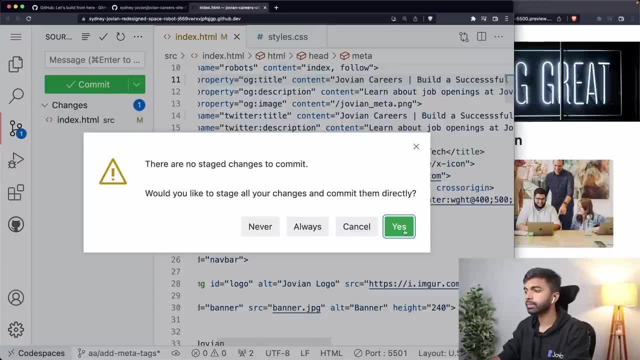 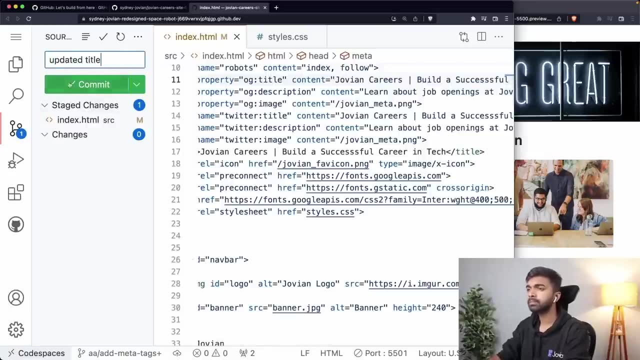 I think I'm happy with the way things are here. So I'm just going to click commit and let me see, I'm just going to stage my changes and let me say updated title and I'm going to click commit and I'm going to publish the. 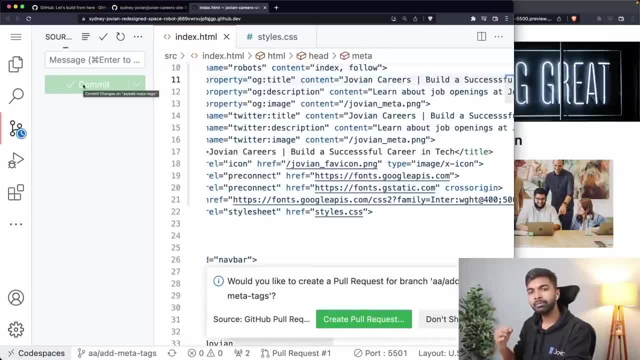 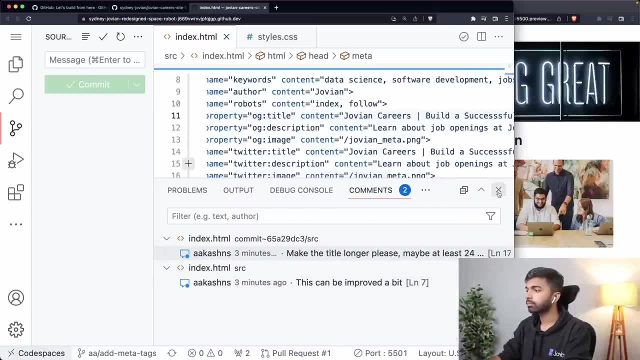 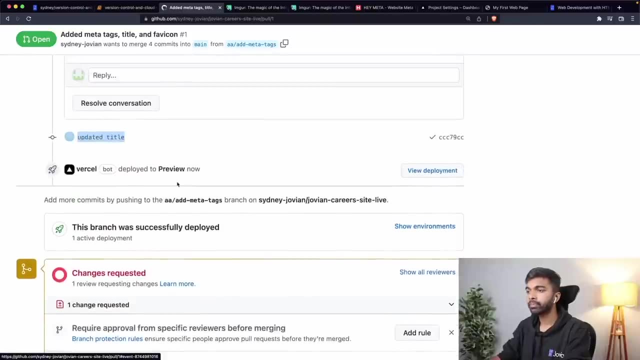 branch. So now, once a pull request has been created, anytime you publish the branch again, the pull request will automatically be updated. Okay, So let's come back here and let's reload this page and you can see that this new commit has been added. 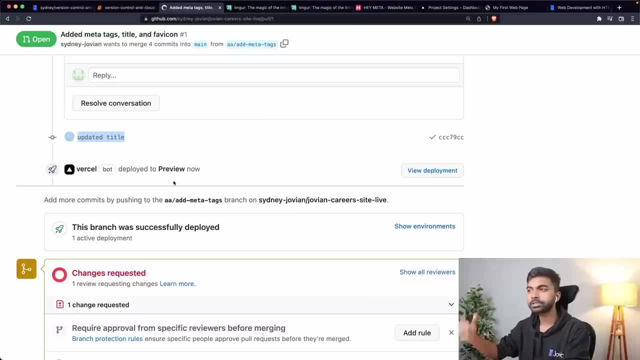 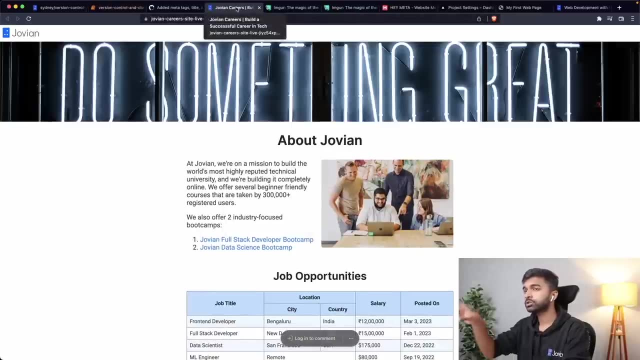 Okay, So it's automatically going to take this new commit and it's going to deploy it. So it's nice like that. So if I go back and check the deployment, this time it has not just Jovian careers, but it has Jovian careers: build a successful career in tech. 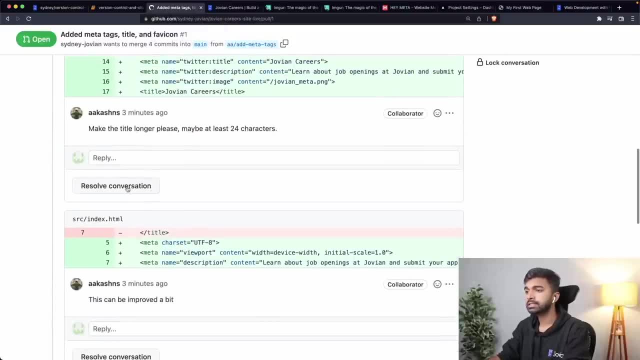 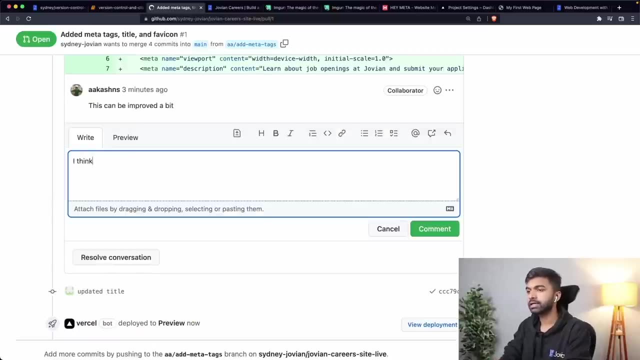 It has the full thing that I've mentioned. Now I can go in and I can say: okay, resolve this conversation, So this is fine. And then here I can say: I think this is fine as it is and I can resolve this comment and 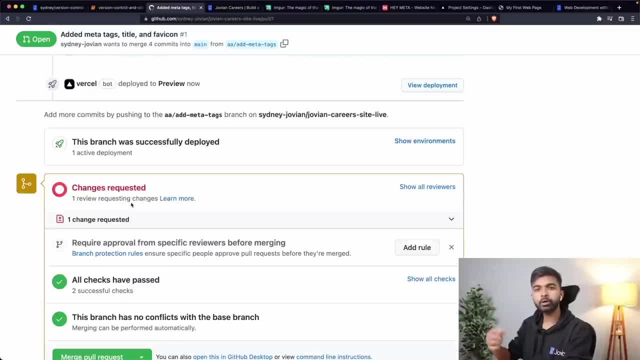 resolve this conversation as well. Okay, So this is what you want to do: You want to resolve all the comments and then the reviewer may go back and make some more comments, And then you resolve those comments and so on, And the reviewer and you both can use the preview deployment to test out your changes. 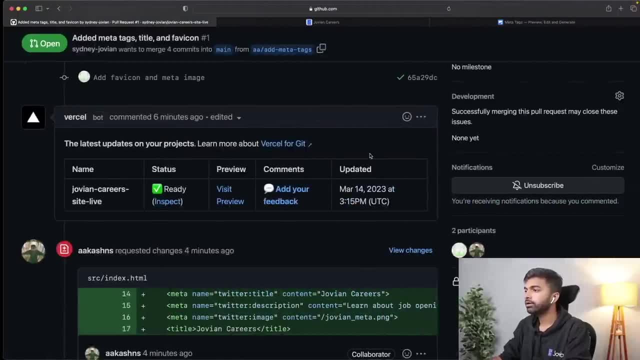 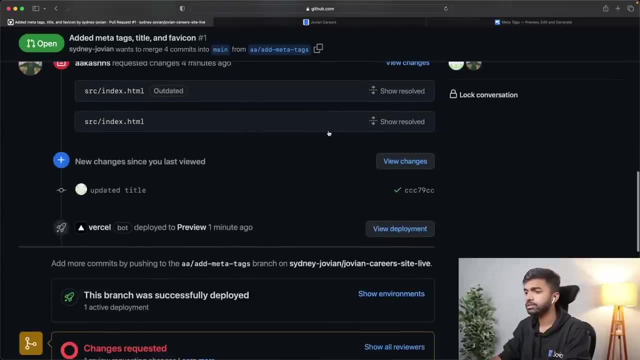 preview the changes live as well. Okay, Now the reviewer can eventually be, can eventually come back later in the day, or maybe the next day, and see that, okay, all their changes have been resolved. So then they can go ahead and they can approve the pull request. 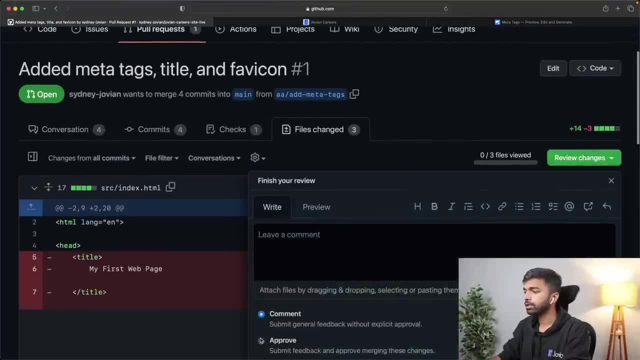 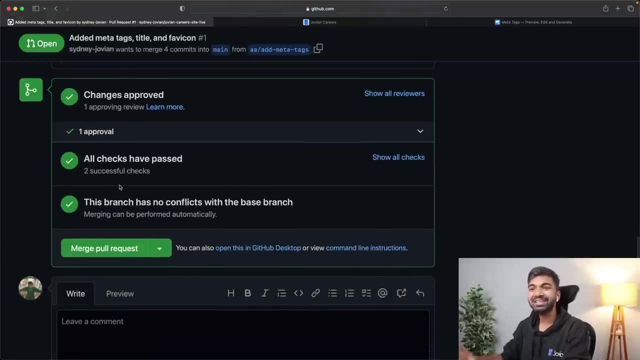 So they can go back into this files tab and they can go in and they they can approve the pull request like that And once the pull request is approved, then the changes can be merged back into the main branch. Okay, So so far. 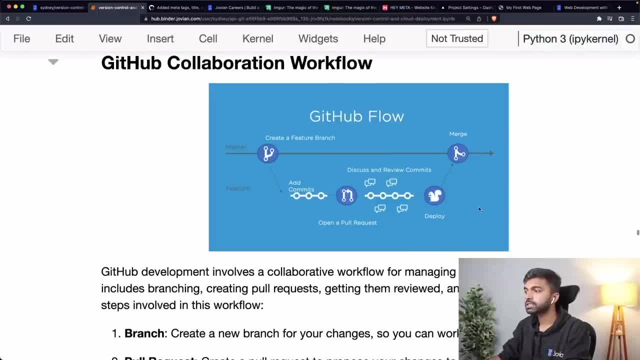 Yeah, So so far we are still at this stage where we have deployed, we have done a done a preview deployment and the pull request has been approved. but to merge it back, Okay, So we come back into the pull review page, the pull request page and at the bottom we 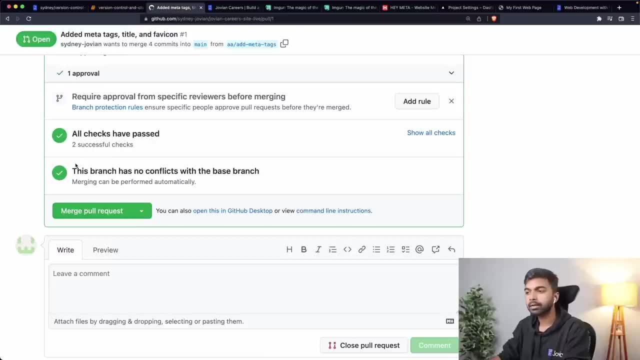 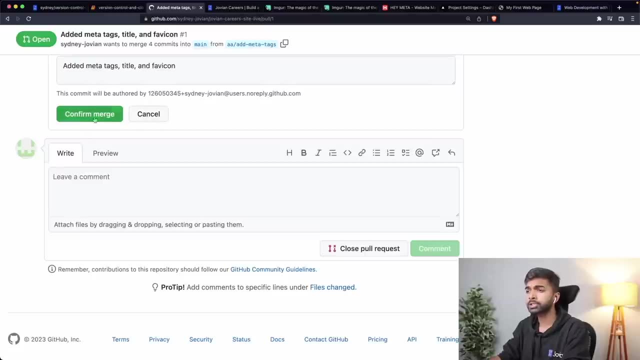 can see that once all the approvals have been have been received and you can set conditions- this at the repository level- then you can click merge- pull request- and you can give it a commit message and a commit details and then you can click merge. 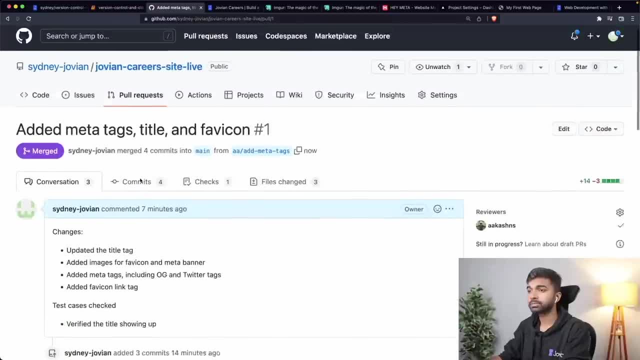 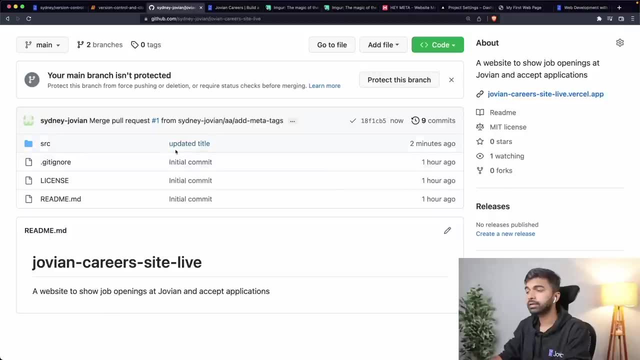 And that is going to now merge this to our main branch. Okay, So now this is merged And now if I come back into the code tab, I see the main branch. Okay, You can see here. now it has this new commit called updated title. 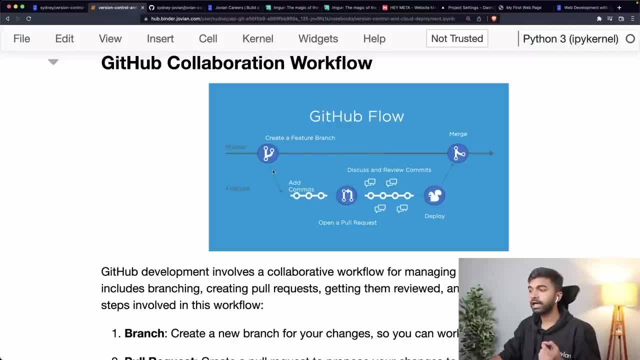 So this is the work, So this is the workflow that we have. We created a feature branch, added some commits to it, pushed the branch, created a pull request. Then we invited a reviewer to comment. the reviewer commented. we made the changes. 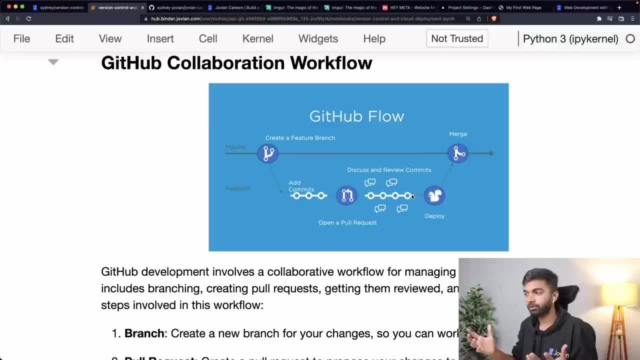 We also looked at the preview deployment which Vercel automatically gave us very kindly, And we made sure that everything was working fine And finally the changes were then merged to the main branch And of course Vercel picks this up again and does another deployment. 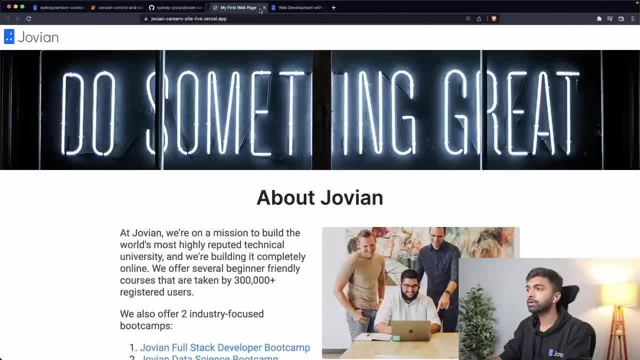 So now, if I go back and just reload the main Vercel page, you can see that now the favicon is updated, The title is here, is updated and I can also check. So there's a place here that you can check meta tags. 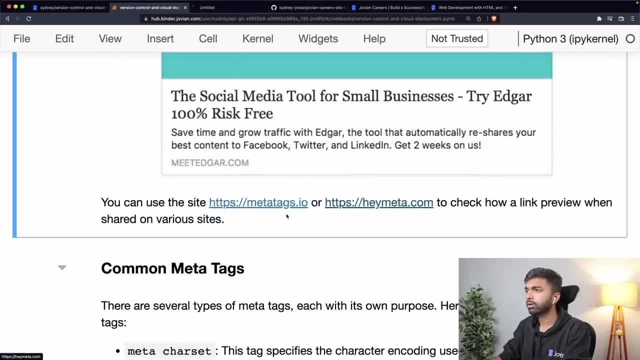 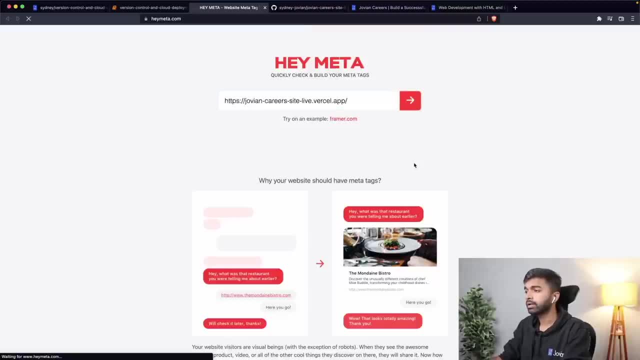 I believe it's called kmetacom. Yeah, So I can also check all the meta tags. now on Jovian careers website: livevercelapp. Okay, So now I can check all the meta tags. So now our careers, Jovian careers website has this nice title that is going to get picked. 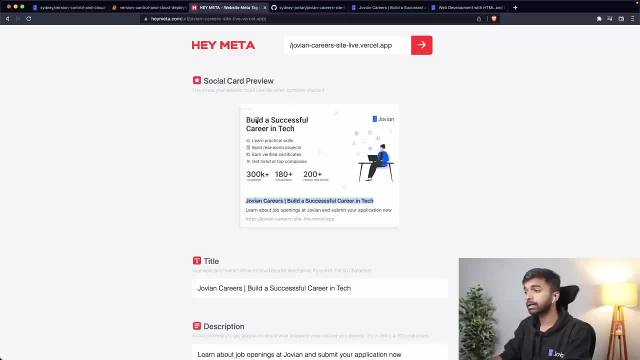 up by Google, Facebook, Twitter, et cetera. It has this nice image that will show up as a link preview When you share this link on LinkedIn or elsewhere, and it has this nice description over here as well. Learn about job openings at Jovian and submit your application now. 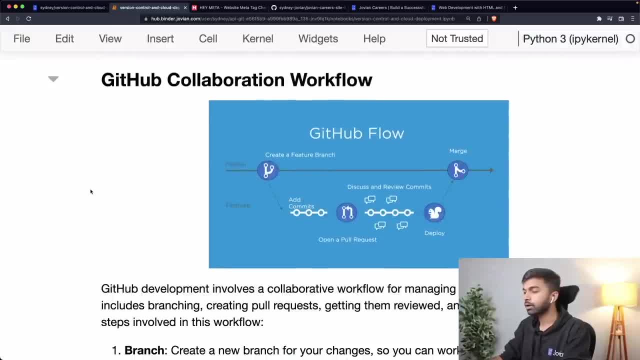 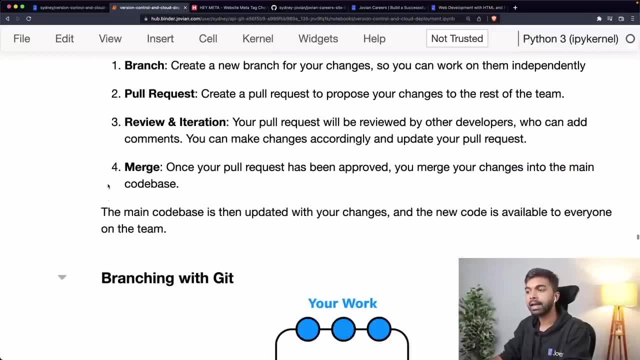 Great. So we learned the. we learned about meta tags, but alongside we also learned about a GitHub collaboration workflow, which is branch pull request: Get it reviewed, Iterate on it And then merge it once you have received the reviews. Okay, 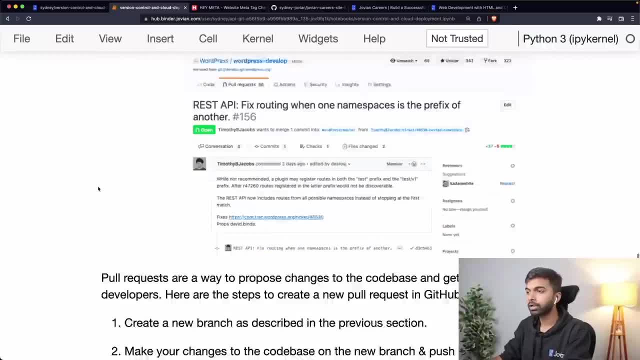 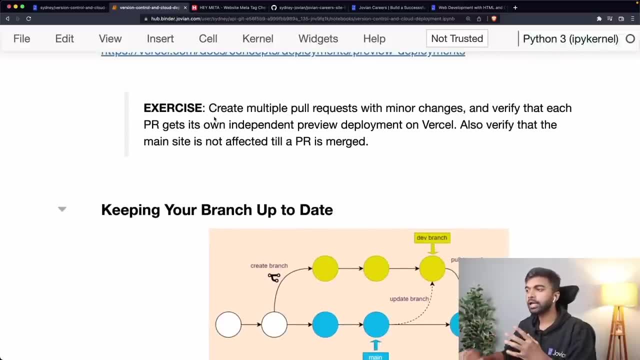 So that's about branching with Git And that is about creating pull requests, And I would encourage you to exercise this a little bit. So create multiple pull requests with minor changes and then verify that each pull request gets its own preview deployment. So if you have five pull requests, they're going to be five preview deployments. 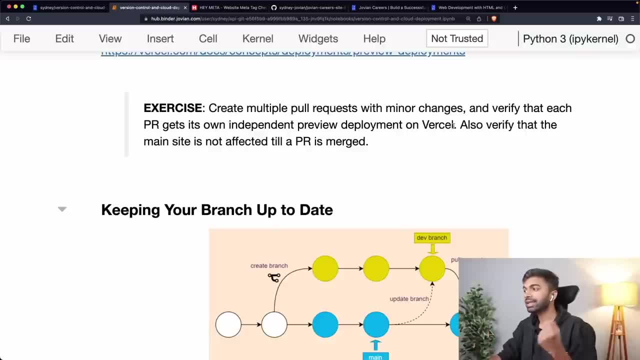 So also gives you unlimited preview deployment deployments for free and then verify that the main site is not affected till a particular pull request is merged. Okay, Also, one thing that you can try to do is try to see what happens if you have two pull requests. 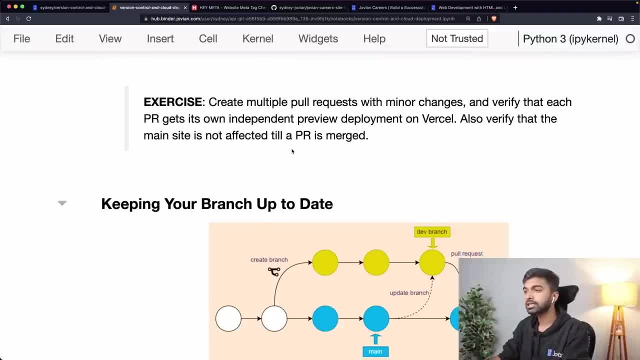 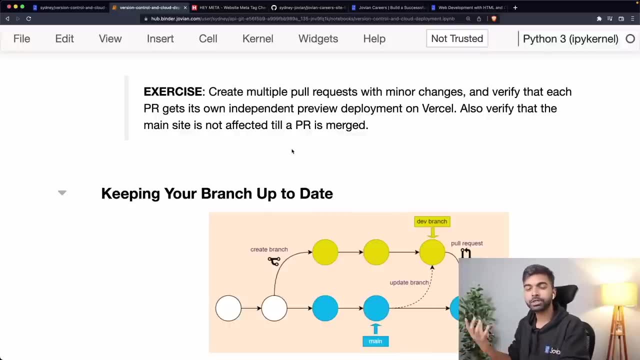 and then you merge one, and then you try to merge the next one. So these are some exercises for you to try out. Git is a very applied skill, So you have to try out all these things. whatever questions you have, just try it within five. 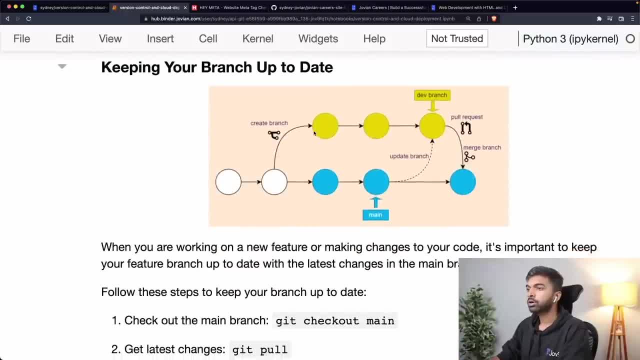 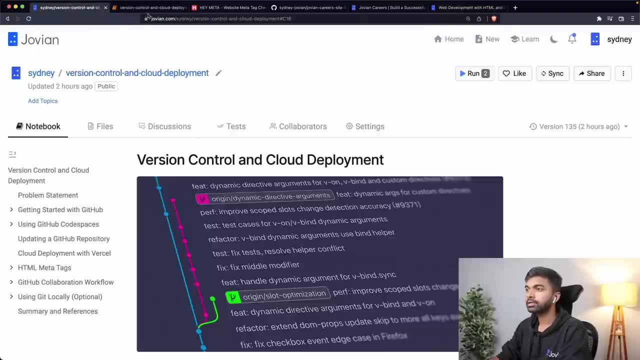 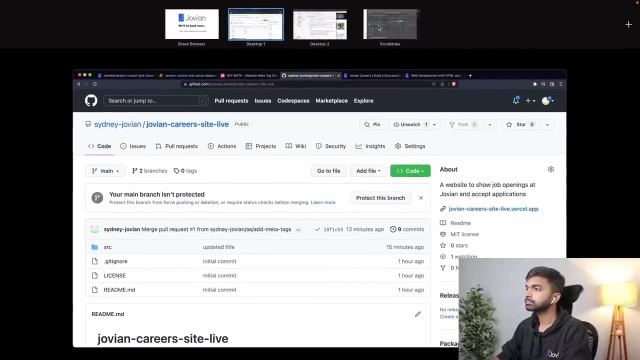 to 10 minutes. You'll actually have your answer. Now let us talk about keeping your branch up to date. So here is a scenario that might happen. We already have two users. Now we have two collaborators. One is Sydney Jovian and the other collaborator is 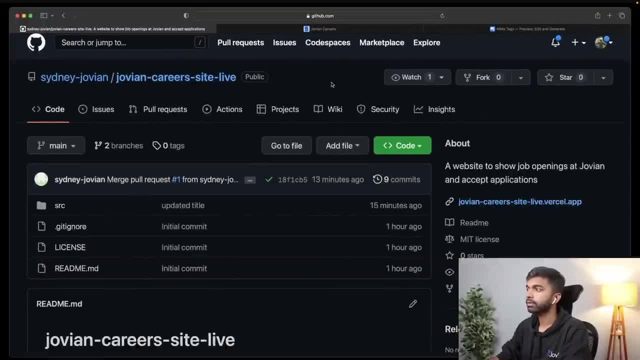 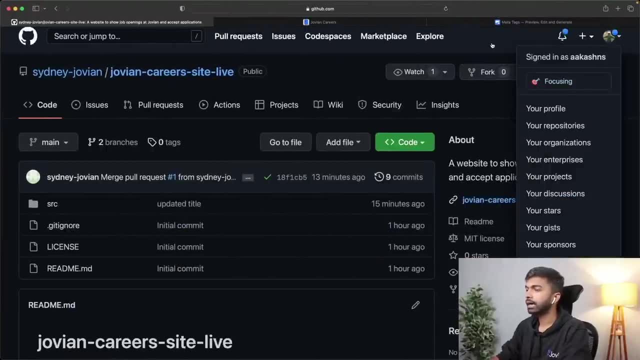 And the other collaborator is Akash NS. So that's why I have these two windows in black and white. So here I am signed in as Akash NS and here I am signed in as Sydney Jovian. Of course, the repository still belongs to Sydney Jovian. 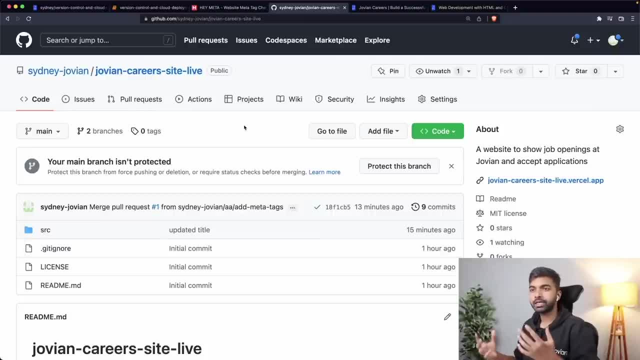 We are both collaborators. Now let us try to make changes in such a way that two people are working in parallel And once changes get merged into main, while the second is still working. Okay, So let's do this. Let us first go into this code. 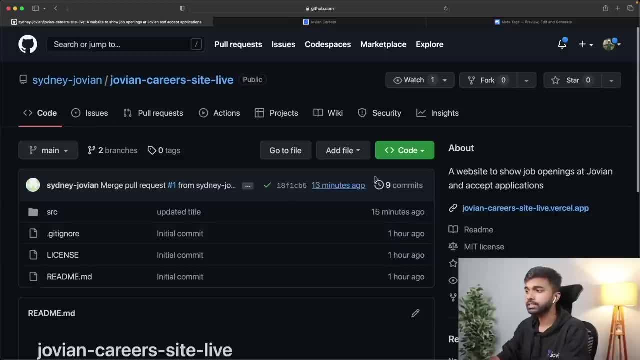 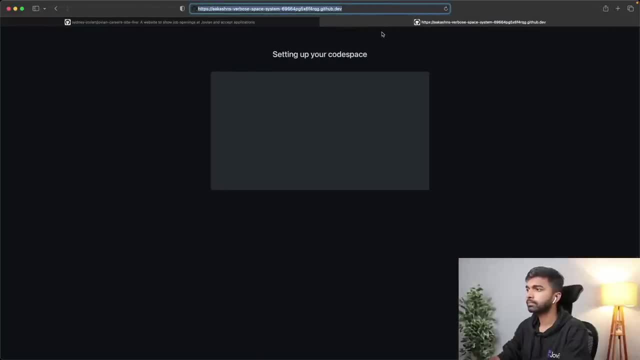 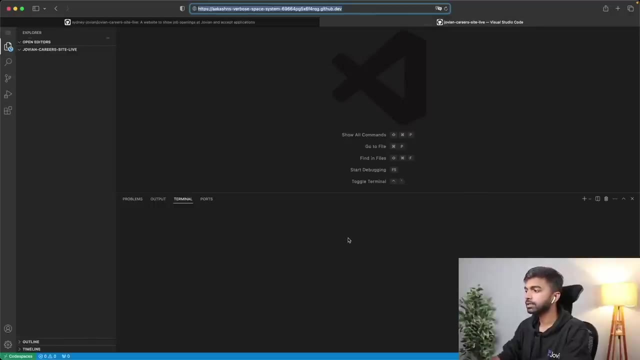 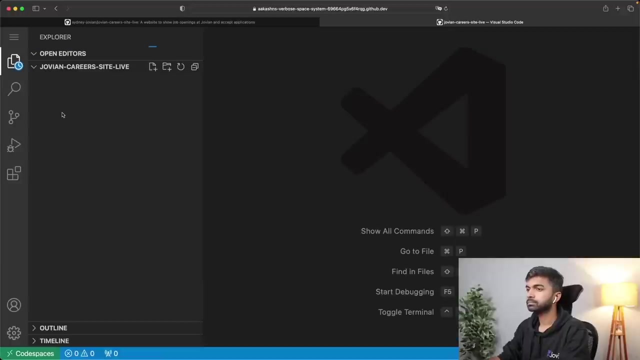 So this is on the user Akash NS and I am going to create a code space to start editing. It's going to take a second or two to set up the code space, But once it's done I should be able to start editing some things here. 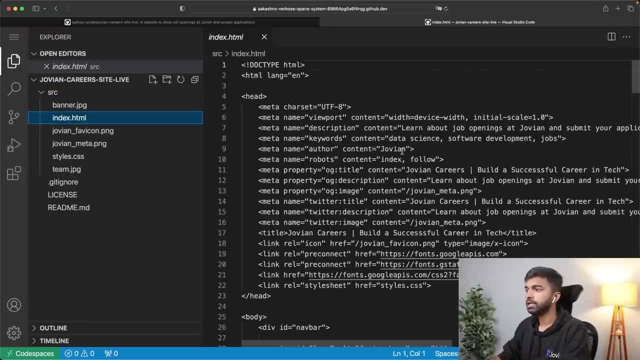 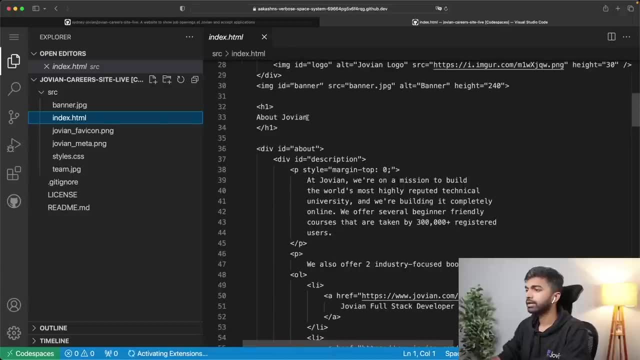 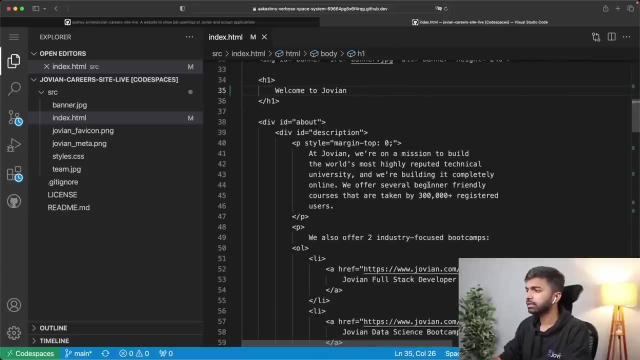 Okay, So inside SRC I have indexhtml and let me just go in here and let me just change this to. let me edit the title again. Let me change this to: welcome to Jovian. Okay, Okay, Okay, Okay. 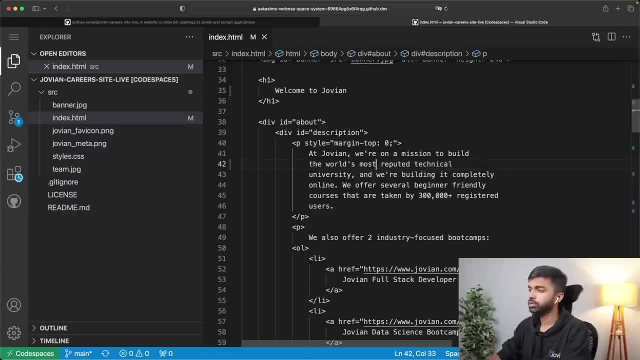 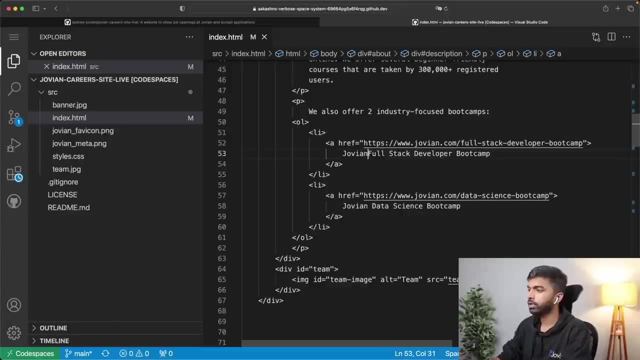 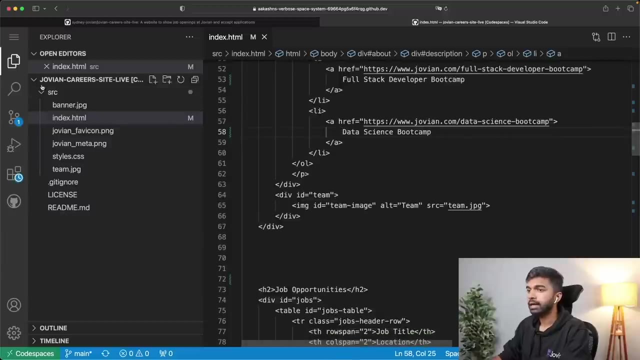 So I have a description. Let me remove highly reputed, Let me just make it most reputed- technical university. So I made a couple of small changes here And let me also remove the word Jovian from the names of the programs. Let us just call it full stack developer bootcamp and data science bootcamp. 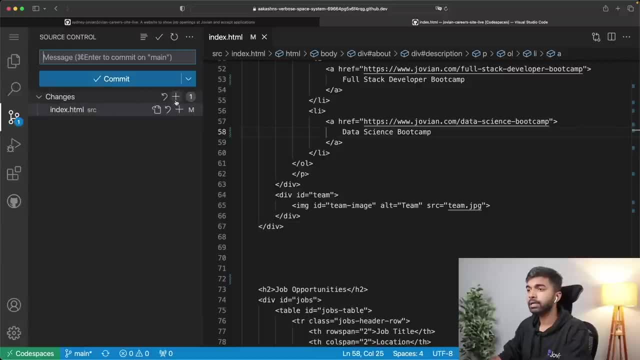 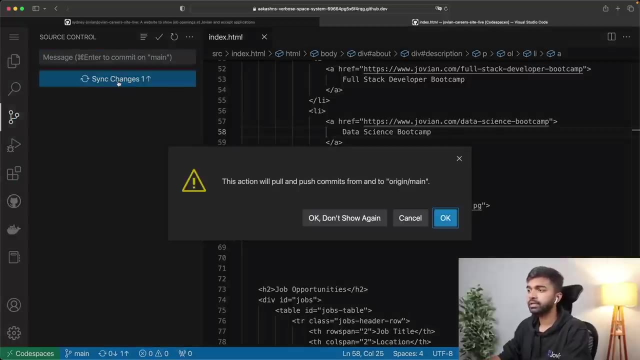 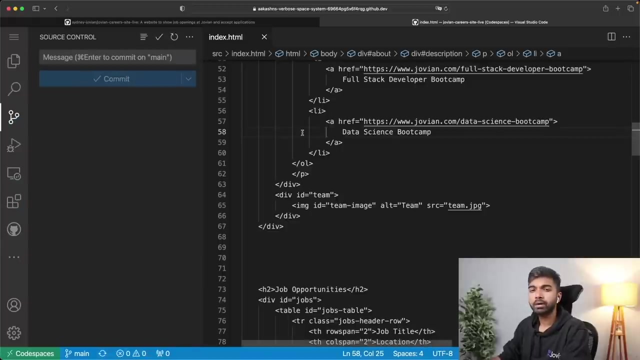 And let me just commit it. So let me go into source control, Let me add the changes and let me say: made some changes to indexhtml And let me commit it And let me sync the changes. Okay, I have synced it, but it looks like I made those changes on main right. 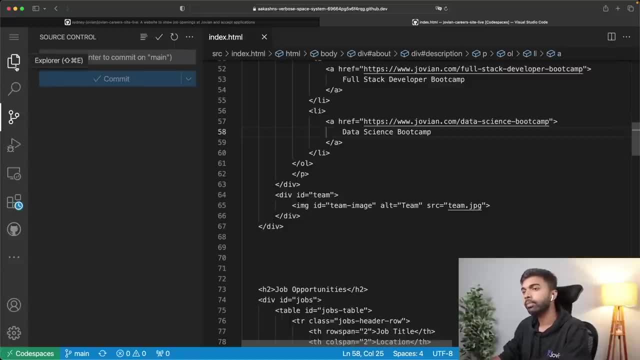 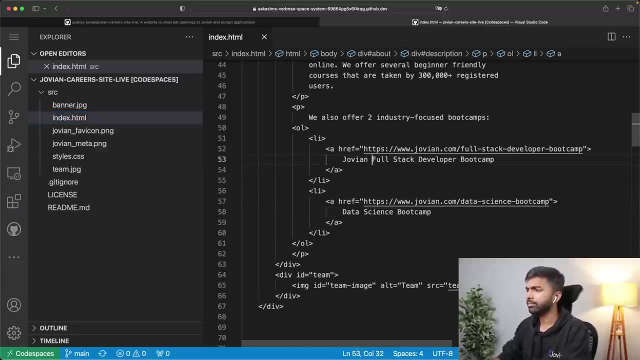 So let me now create some more changes and let me make those on a branch, because normally this is not something we should be doing. We should be creating a branch, but let me add back. let's say, let me add back the word Jovian here. 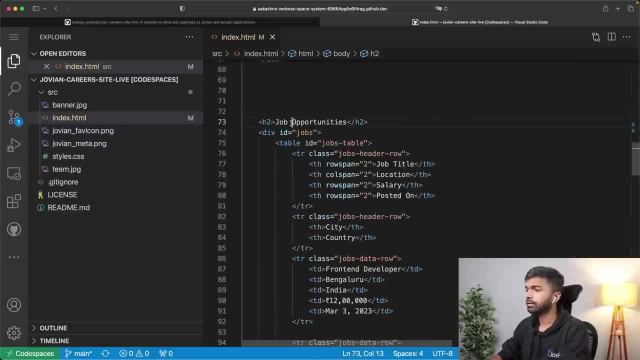 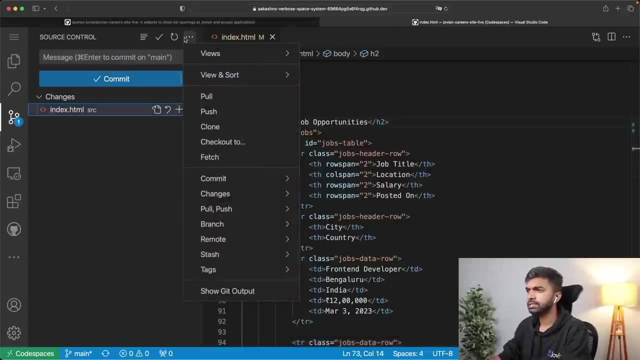 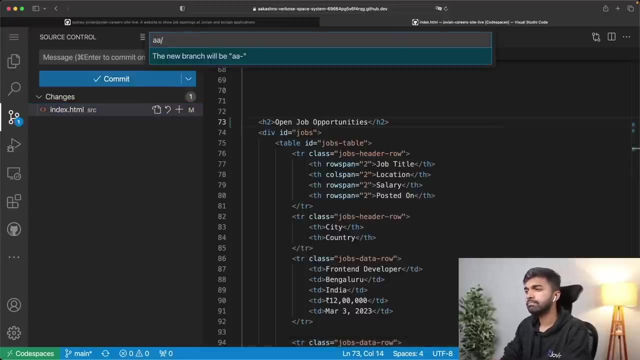 Let me add back the word Jovian here, And let me add the word open job opportunities here, And this time I'm going to first create a branch. So let's see, let me create a new branch. Let me call this branch open job opportunities. 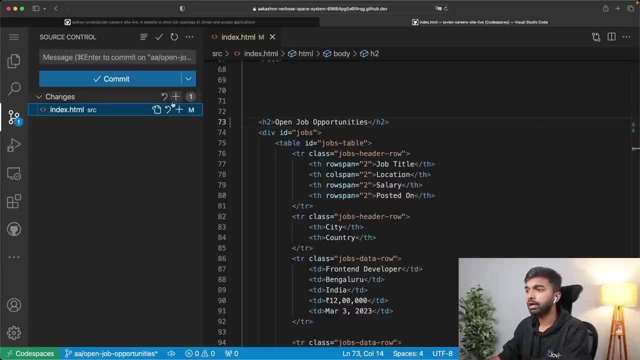 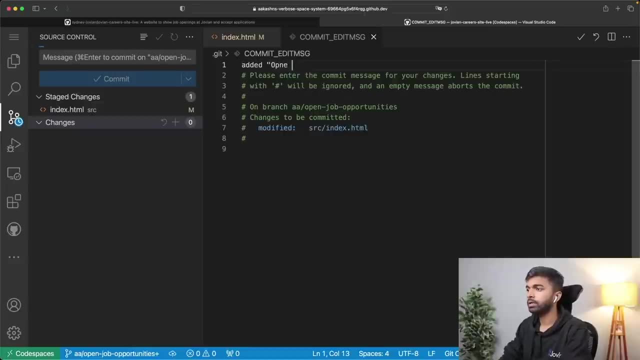 And now the branch has been created and now I'm on the branch, Now I can add my changes to the to my branch And let me commit them. Okay, So I did open job opportunities, okay, And now let me publish the branch. 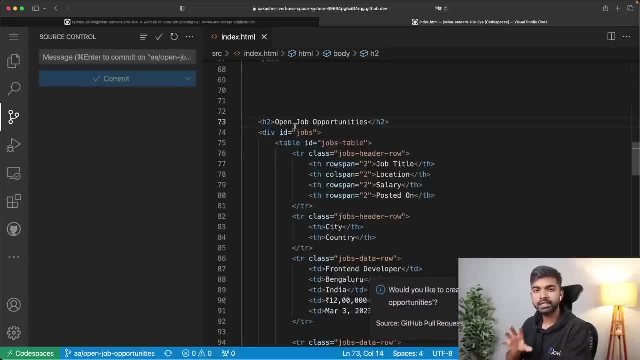 So what I've done now is I have made some changes on main and that will just go out to everyone for sure, But then I've also created a branch out of main which I'm going to then create a pull request on. So I can then come back here and it looks like: okay, this new branch has been pushed. 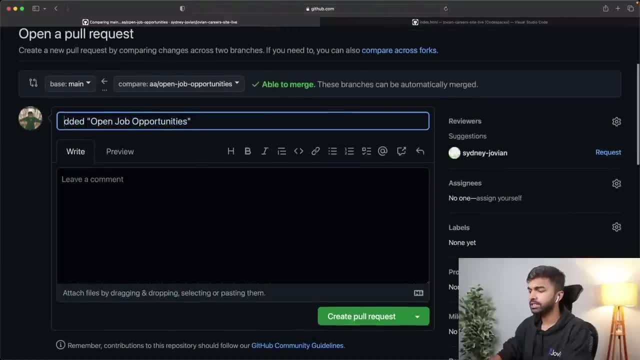 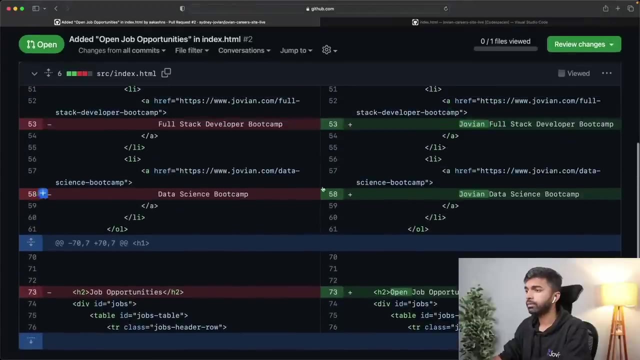 Let me click compare and pull request And let me just say: added open job opportunities in indexhtml And that's the same description. for now, Let me create a pull request And the changes that have happened here are simply well, from the main branch, I have 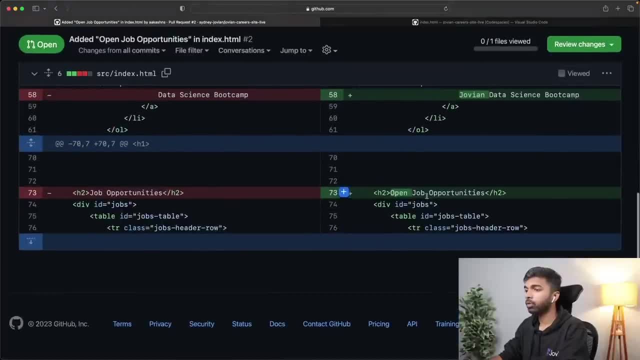 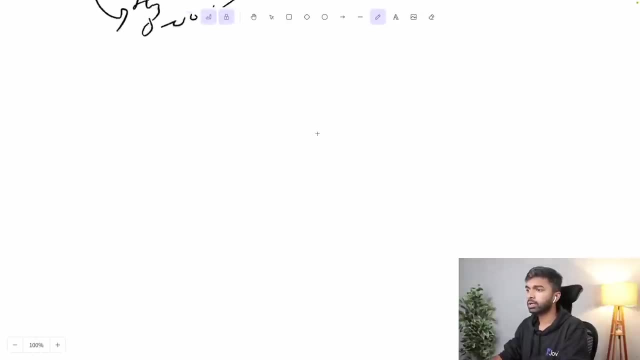 simply removed, added the word Jovian back and I've added open job opportunities here. Okay, So just to show you what happened, What we did was we had the main branch And then from the main branch we made another commit. 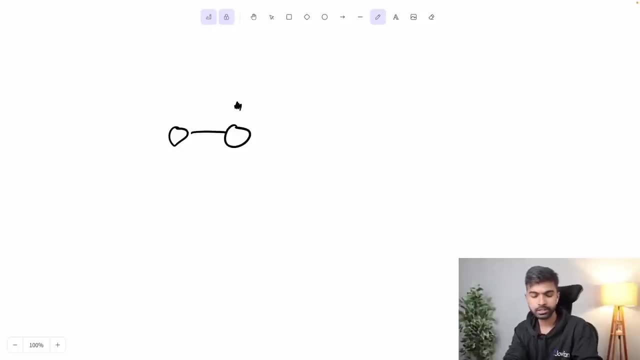 So we made some changes onto the main branch. This was done by our consciousness, So this was the main branch. Then we branched out of the main branch and made one commit And of course we've got to make multiple commits on that branch. 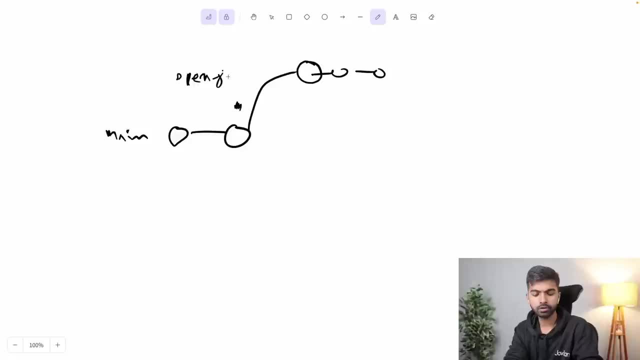 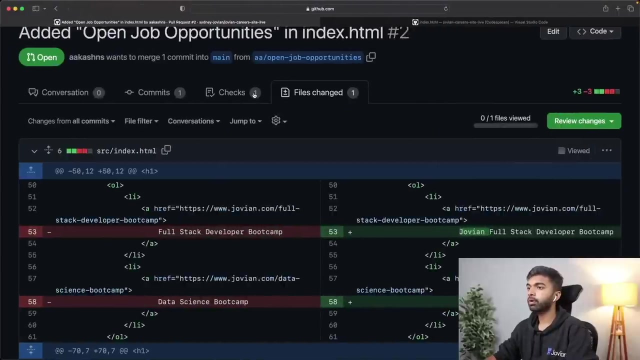 So this branch is the open job opportunities branch, right, And this branch has been made by Akash And we have set up a pull request for this branch as well, right? So let us call this pull request one. Now, we have set up a pull request, pull request one called added job opportunities in indexhtml. 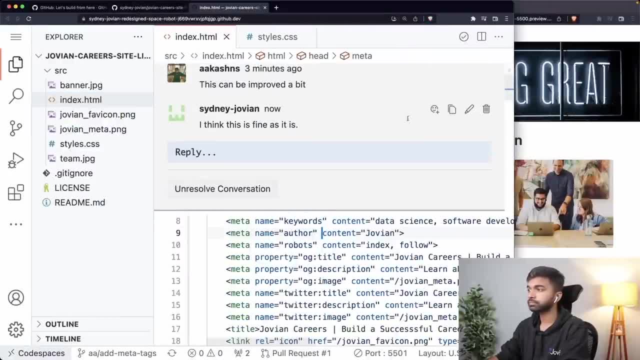 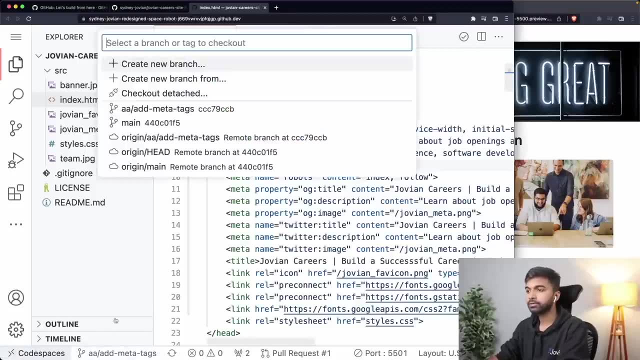 Now let us come back to Sydney Jovian, Okay, And let us go back here to the main branch first. So there is a selector here that I can use to go to the main branch. Let's say here: I've just checked out the main branch. 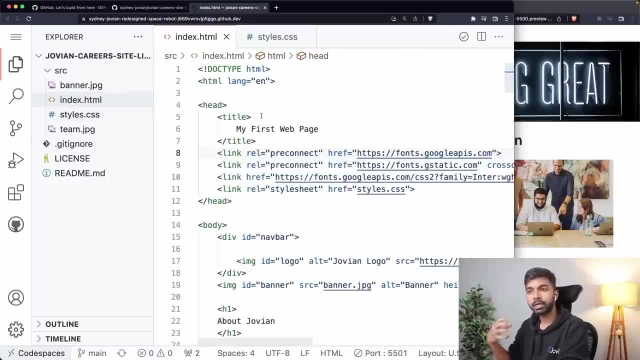 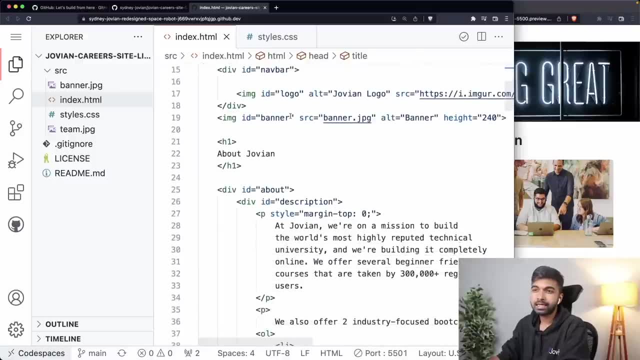 Okay, Now the main branch on Sydney Jovian is a little bit behind my old branch, the branch that has been created by Akash NS. So let's say Sydney forgot to pull the latest changes before, before working on a new change. 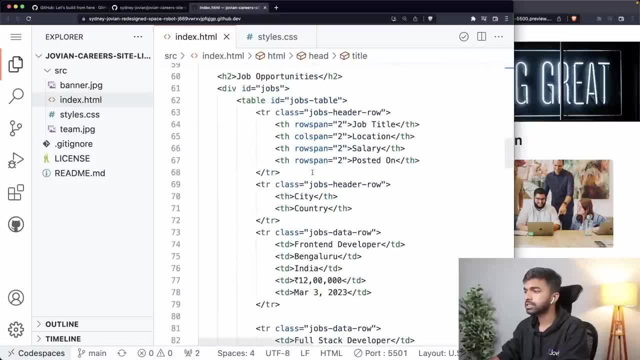 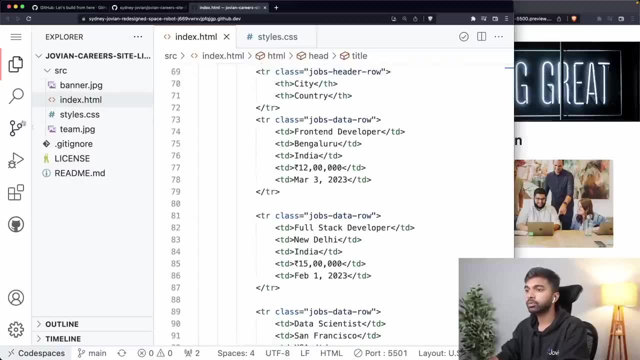 right, Let's say Sydney is working on some changes about related to the dates of the front end developer, backend developer, et cetera. So what Sydney does is creates a new branch to make his changes. So I'm going to say branch. 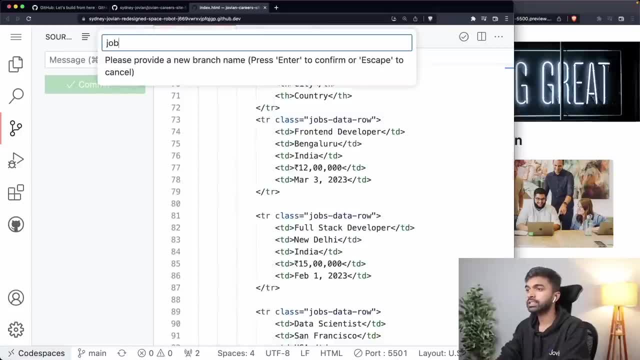 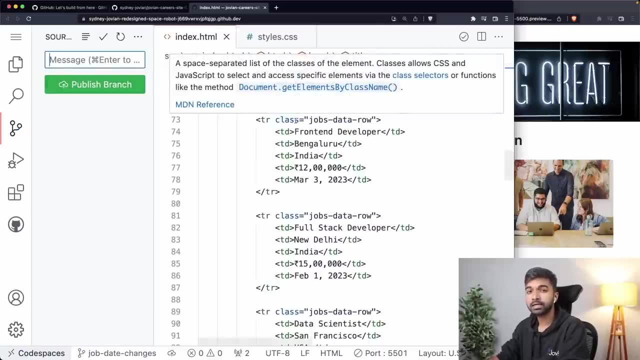 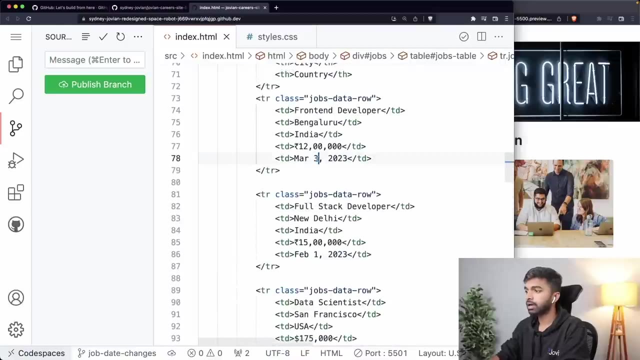 Create a new branch. And let me just say job date changes and create this branch. The branch has been created by Sydney for his work And now Sydney is going to make the changes to the jobs. Let's say this is March instead of March 3rd. 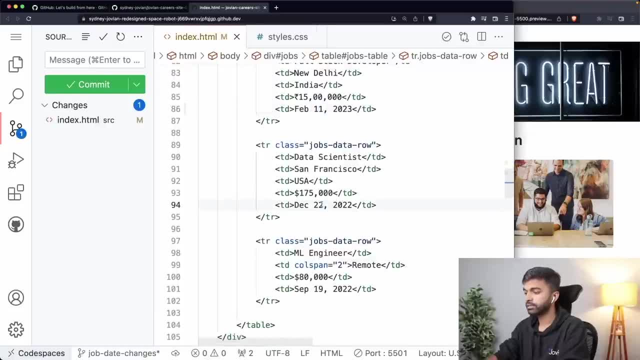 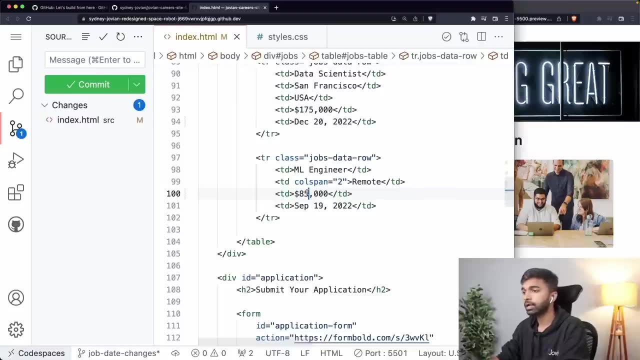 This is March 13th Instead of Feb 1,. this is Feb 11 instead of December 22nd. This is December 20.. And here we change the salary to 85,000.. Okay, Okay, And now let me commit these changes into the branch. 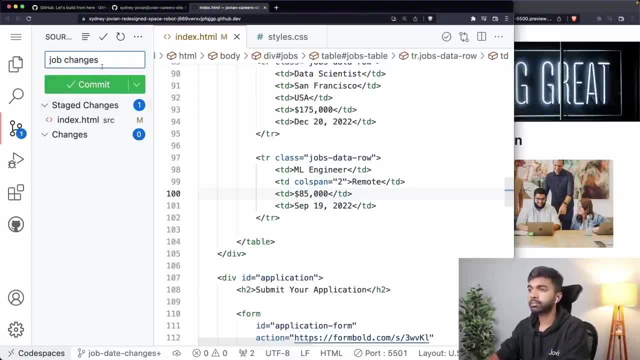 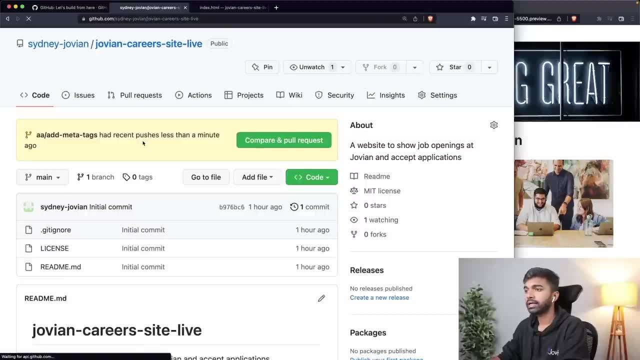 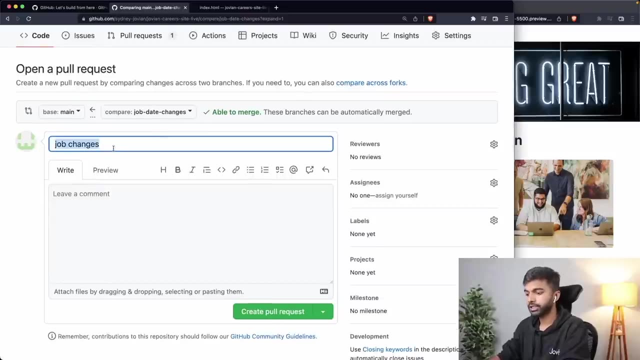 I've staged them. So job changes and commit and let me publish this branch, And now let me again come back here and let me create a pull request. Okay, So once again, these are job changes, so job date changes, and this is again something. 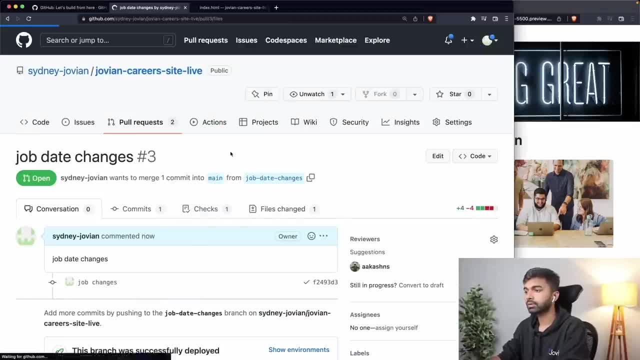 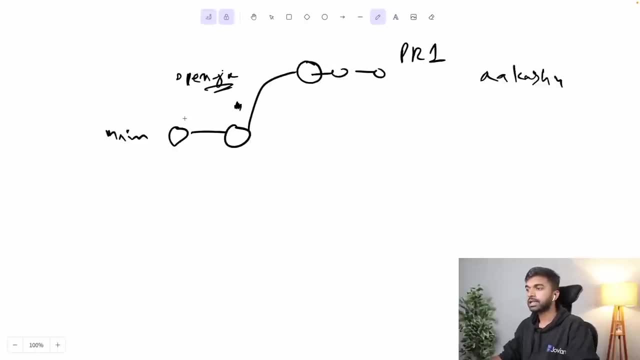 that I would want to merge. Okay, And the only changes here are the changes within the dates. So let's once again recap what's happening here. So your occasion is has first made a change to the main branch itself and pushed it, and 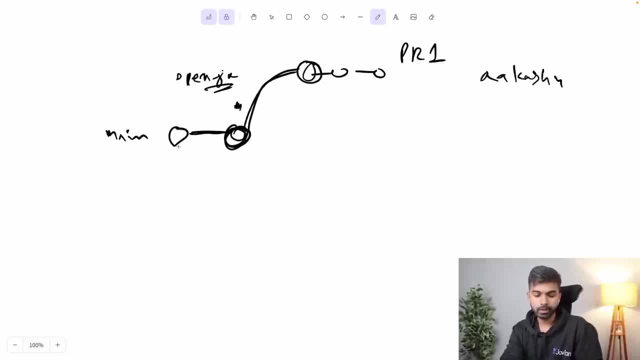 then created a new branch and created a pull request on top of it. Then Sydney Forgot or did not have a chance to pull the latest changes on main. So Sydney created a few changes from the last version of main and then made a couple of. 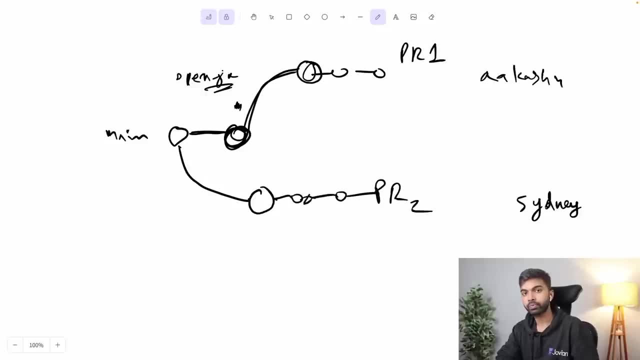 comments, let's say, and then set up a pull request. Let's call it PR too. Okay, So already things are a little out of hand. Sydney is Sydney's main branch. on his own computer is a little bit behind, and our caches? 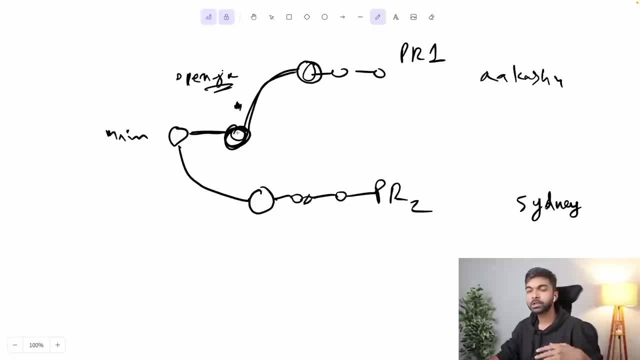 main branch is a little bit ahead And of course this is also the main branch on GitHub itself- So that's where you have a origin- has its own main branch, but Sydney has its own main branch, which is a little behind. And now there is this pull request. 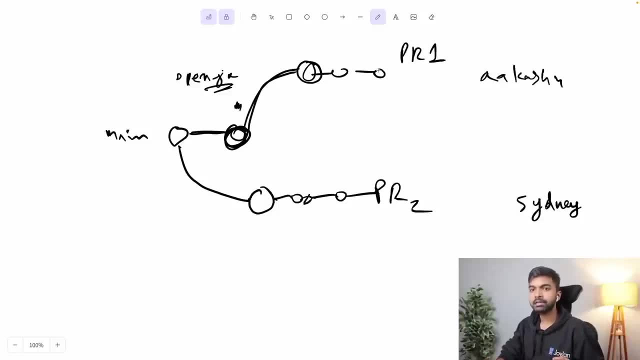 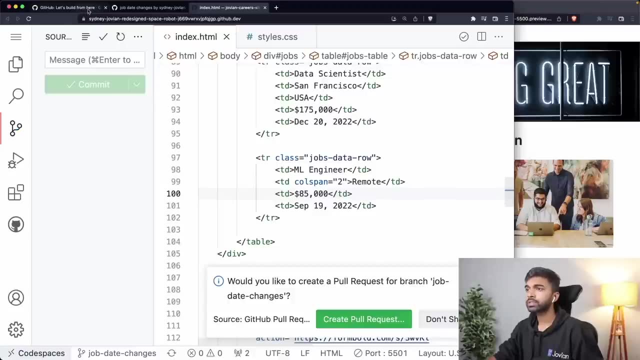 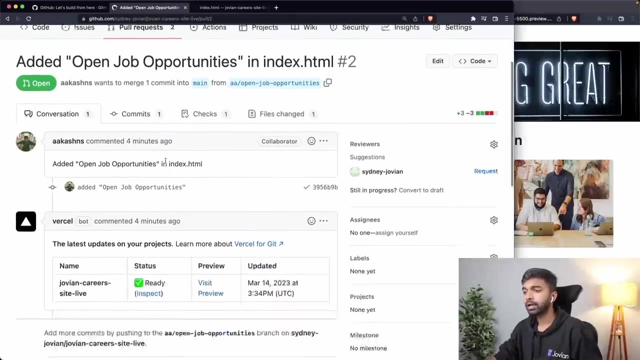 And now one of these pull requests is going to get merged. Let us say the pull request number one gets approved. Let's say somebody on the team goes ahead reviews the pull requests that are all present. So let's say they go into the pull request created by our caution is and they go ahead. 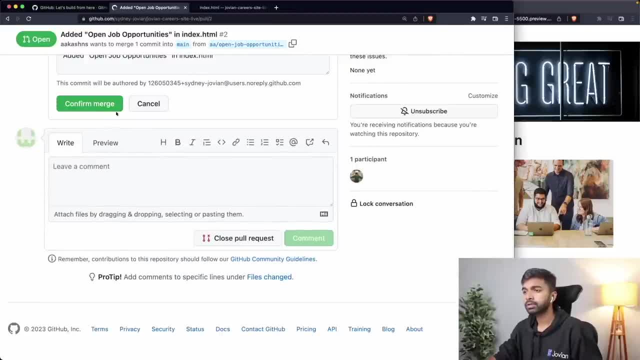 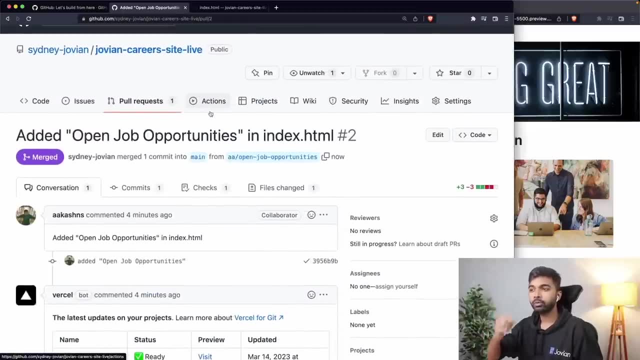 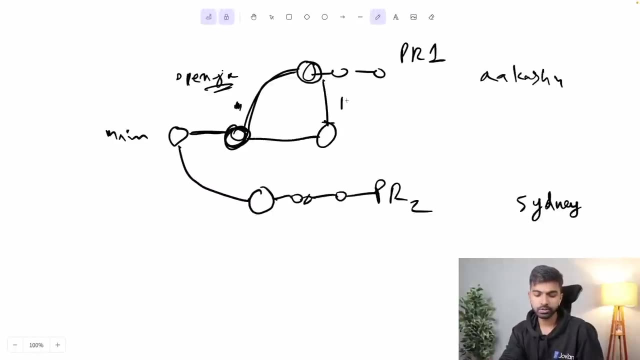 and approve the pull request. Okay, So they just approved it And they just merge that pull request. So now what has happened is that our cautious changes have gone into master. So now we are at the situation where this pull request has been merged back into master. 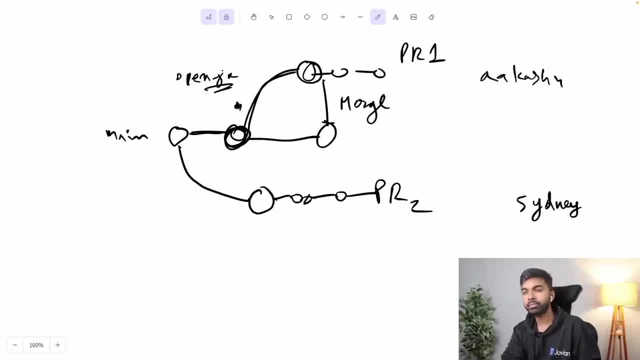 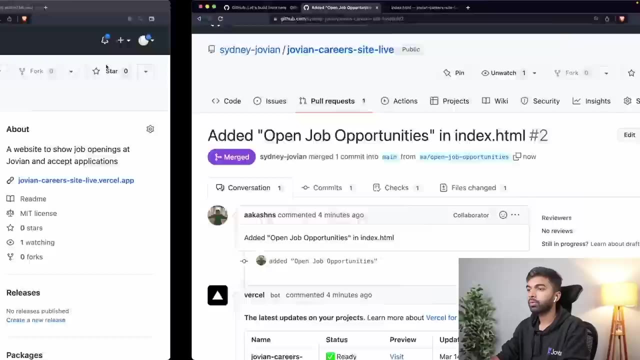 And, however, this pull request is still tracking the old main branch. So now what we need to do is we need to update this second pull request to show changes based on the new new main branch. Okay, So here's what we need to do. 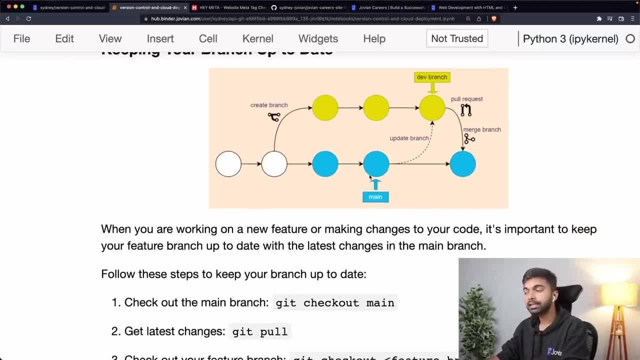 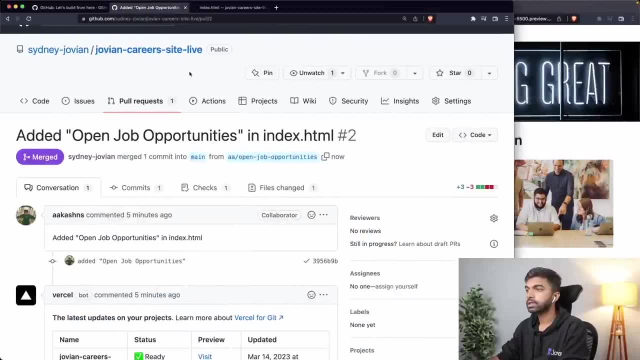 We need to take the changes in the main branch and then incorporate them into the currently open pull request. How do we do that? Well, here is a step by step process. Once we check out the main branch, then we pull changes from the main branch. 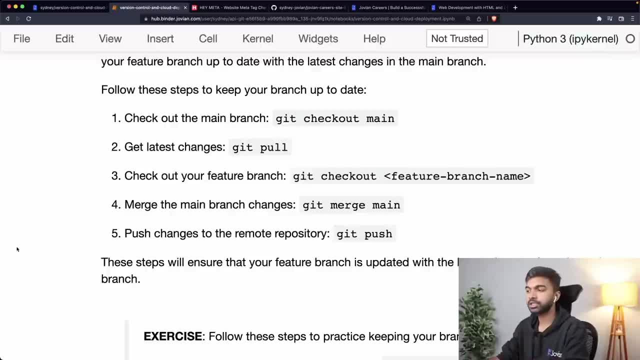 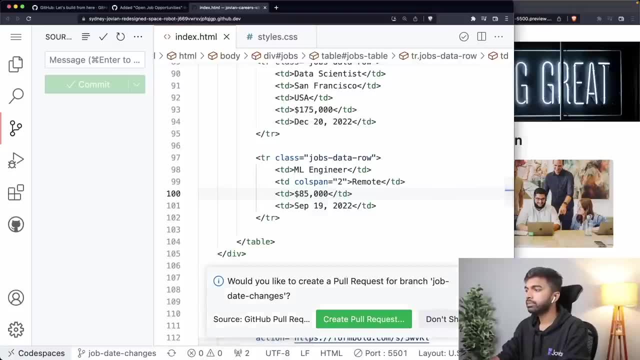 Then we check out the feature branch and then we merge the main branch and then we push the changes. Okay, So we'll do it step by step. Okay, So let's see if this makes more sense. Okay, So now I am here on Sydney's branch and on Sydney's I'm on Sydney's pull request branch. 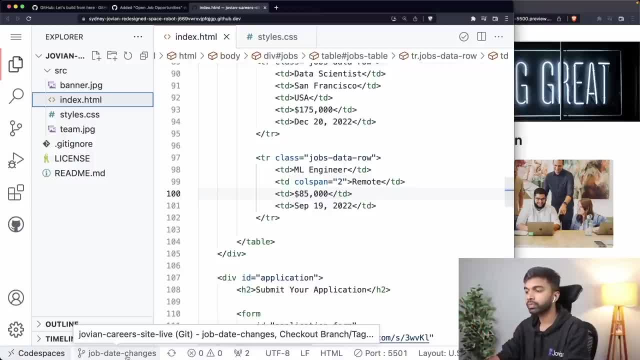 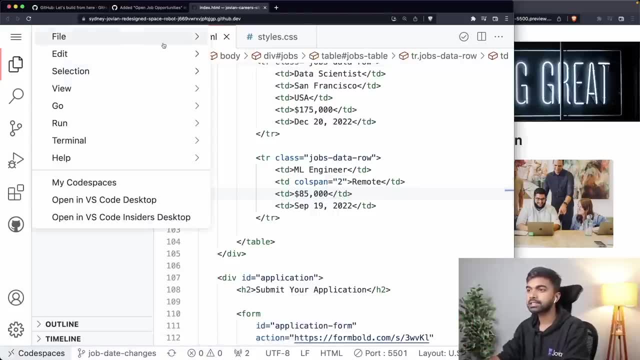 So I'm on the branch which Sydney has created for pull request number two, and this is based off of a main branch which itself is very old. Okay, So I'm going to show this on the terminal, but you can. you can do the exact same thing. 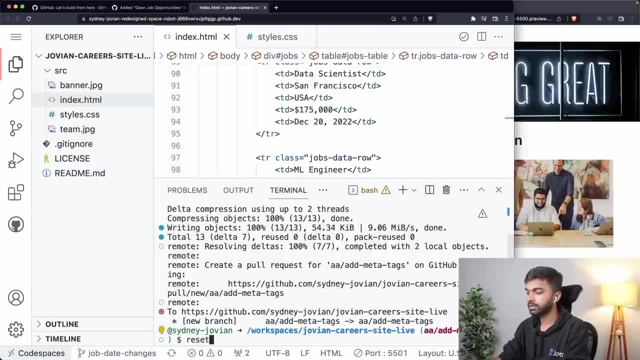 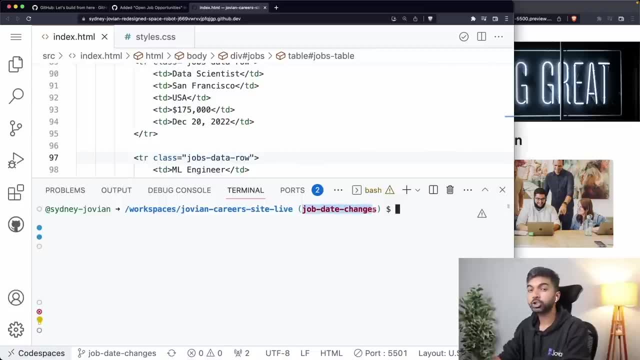 from your, from the user interface as well. So first I am going to- So I'm currently on the branch job date changes. I'm going to switch to the main branch, So get checkout main. okay, By typing get checkout main, I have now switched on Sydney's code space. 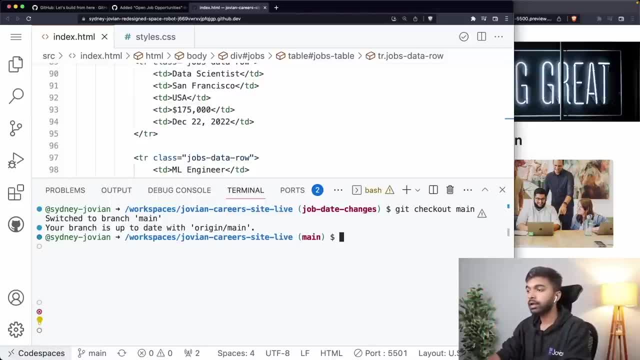 I've switched into the main branch on Sydney's code space. Now, of course, Sydney's code space main branch is behind the main branch on the server. We already know that because one direct comment was made and then one pull request was merged. So I can do that. 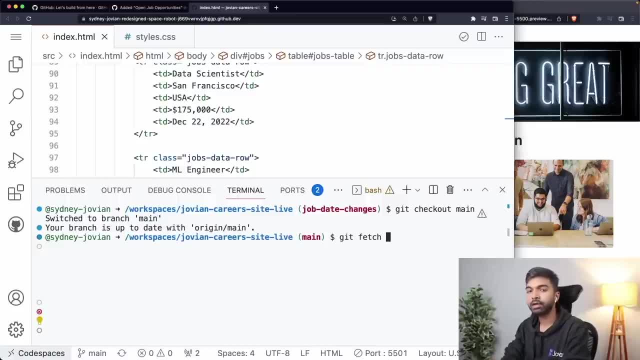 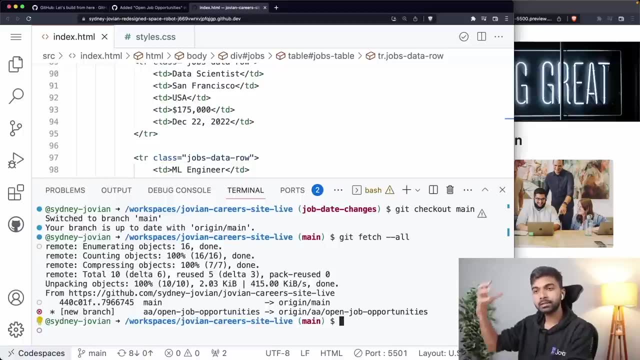 So I can do um. the first thing I can do is I can do get fetch minus minus. all What that does is that fetches the changes that are there on the remote, but it does not apply them yet, So it does not pull the changes. 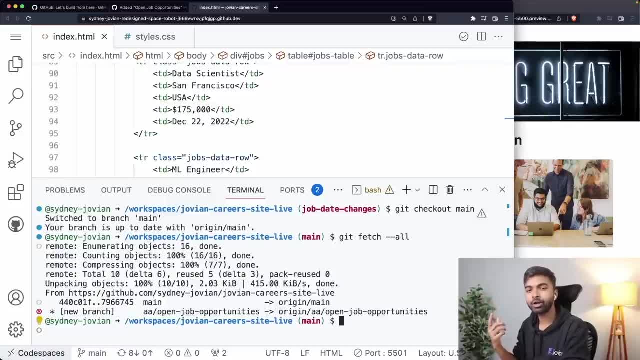 It simply fetches information about the changes. again, more terminology, I know, but we right now, what we know is we we have now fetched information about what are all the branches that are present on the remote server and where are the where. 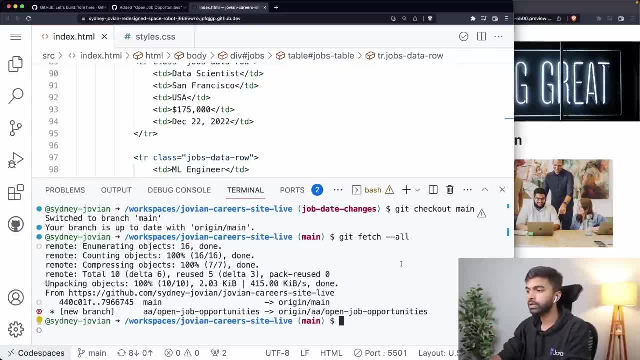 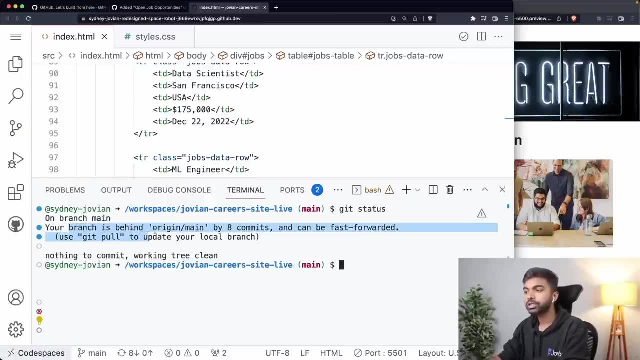 are they compared to the branches that are present on this server? Okay, Let me know reset and let me type get status again. And now I can see here that your branch is behind origin main by eight comments. So it looks like I'm fairly behind because a bunch of other pull requests emerged. but 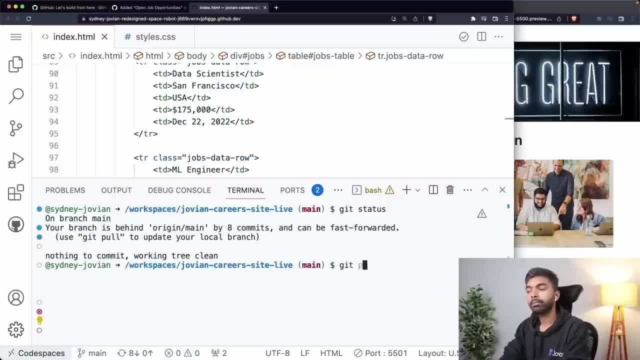 here's what I can do. I can say: get full origin main. So now what I'm saying is that I have my local main branch, which is a little bit behind, And then there is the server, This origin main branch, which is ahead. 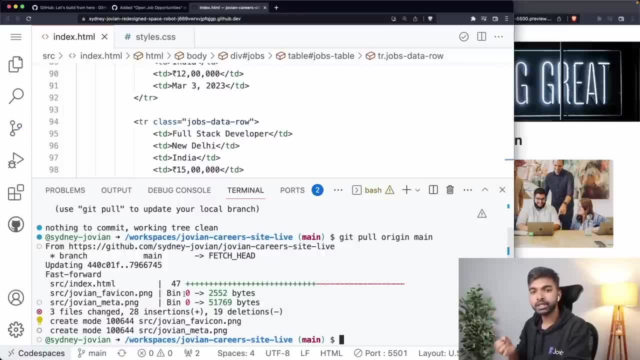 If I type get full origin main, then all my changes are going to get my. my main branch is going to get up to date with the origin. Okay, So what has happened now is that Sydney is local. copy of the main branch has become up. 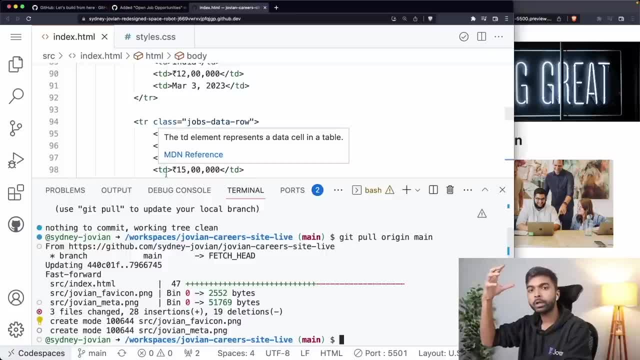 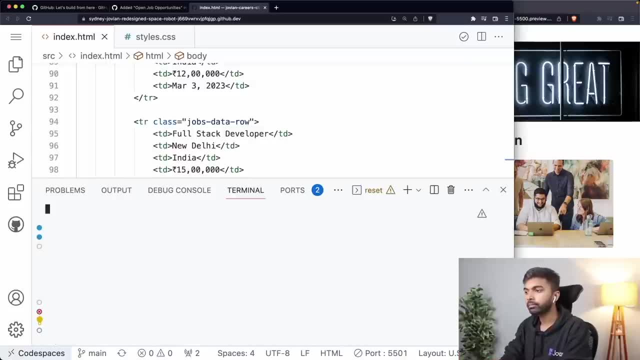 to date by a with the main branch on GitHub. Okay, That's fine. Now let us come back to our Job openings branch. So I can just type get branch to see the names of the different branches that are available and I can switch to the branch. 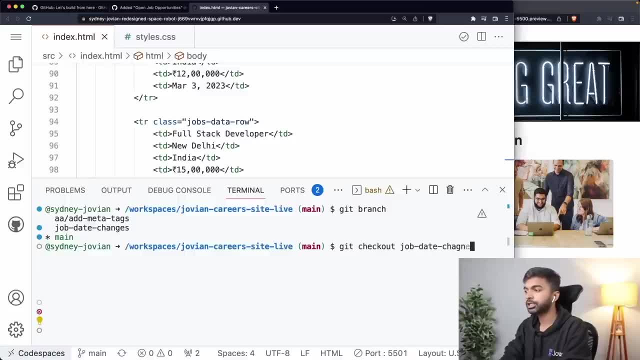 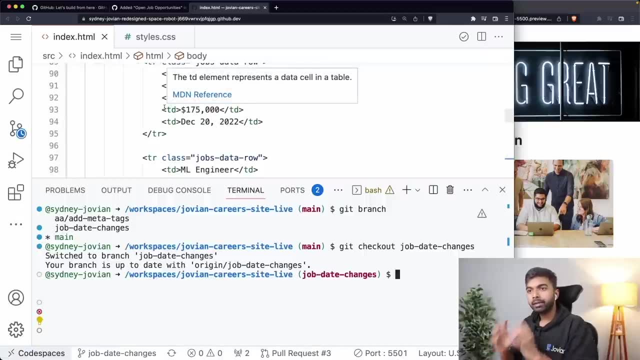 So I guess I get checkout job date changes. Okay, Now I've checked out job date changes. The trouble is, my local main branch is now up to date. My local main branch is now up to date with what. what is there on GitHub, but my job. 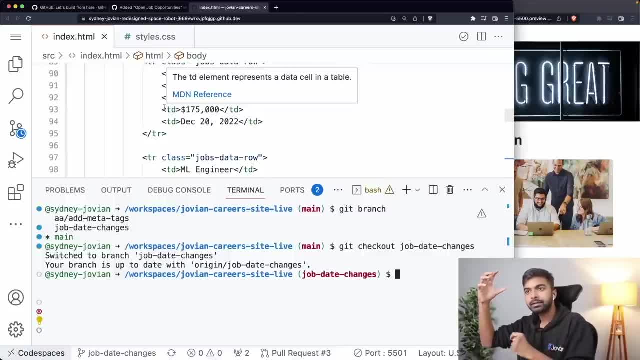 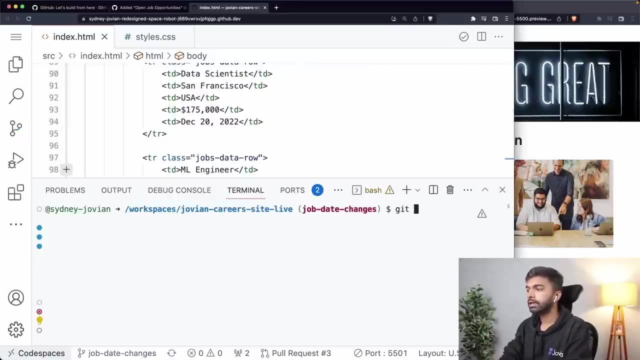 main branch, but my jobs feature branch, Which is still pointing to that old main branch or that old main commit. Okay, So what I need to do is I need to pull in these new changes into my job branch. So now we do get full or not pull. 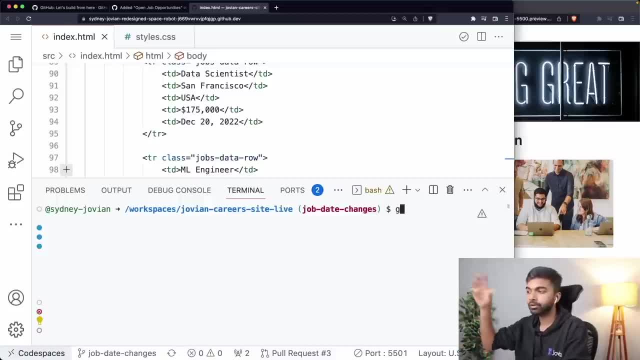 Well, actually we need to merge in these new local main branch changes into the job branch. So we say, get, merge main. What we're telling Get Now is that I'm on this job date changes branch. Take the latest changes from the main branch on my computer, which is already tracking. 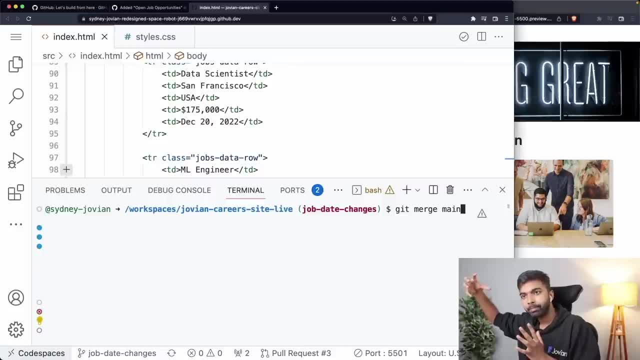 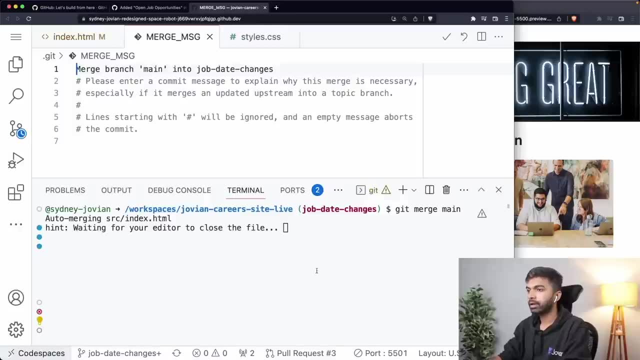 the latest changes from from GitHub and bring all those latest changes back into my feature branch. Okay, So I type get merge main and this will ask me to then type a message. So I'm just going to say merge main into job date changes. 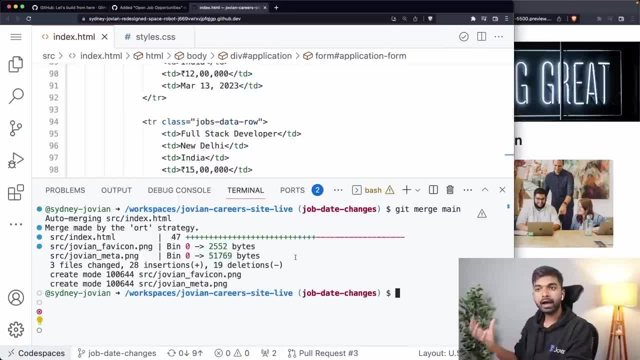 And And now, magically, what it has done is it has taken all the changes that have been made in the main branch on GitHub And we first pulled that into the main branch on our computer. Now all those new changes have been put into our feature branch, which is job date changes. 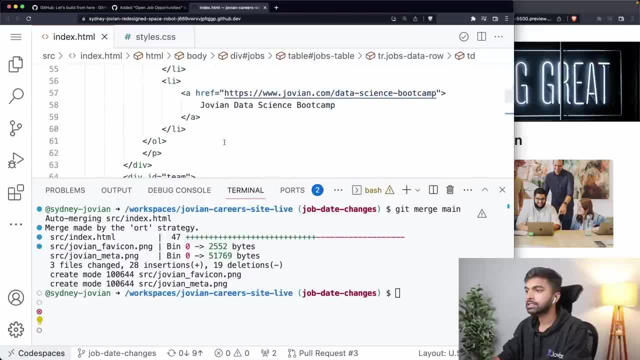 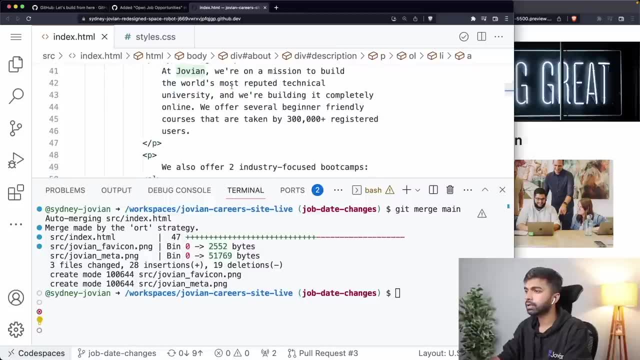 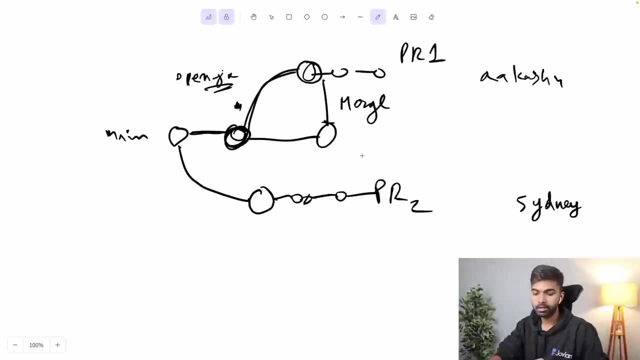 Okay, And you can verify that. here is how you can verify that. you can see that we have Jovian data science bootcamp mentioned here. So that is there. You can see that we have Uh most reputed technical university. So all the changes that were made by Akash I have now been incorporated. 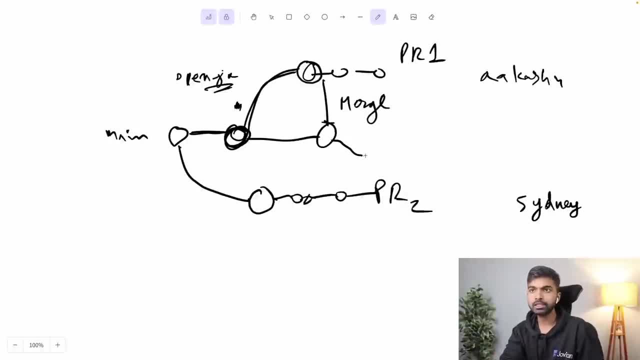 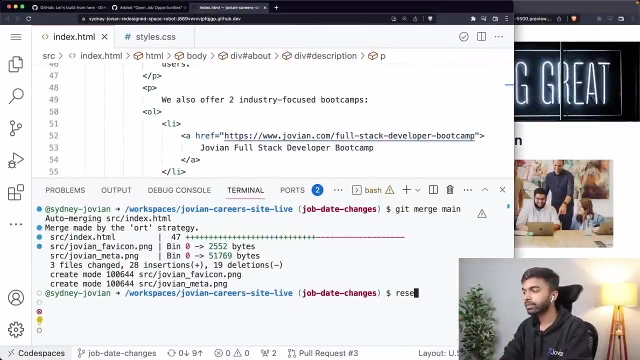 So what we have done essentially is we have taken the changes that have come newly and we have incorporated them into the second pull request branch. Okay, One last thing to do here is that these changes are still local on our code space, So I need to push these. I need to say get, push it to the pull request. 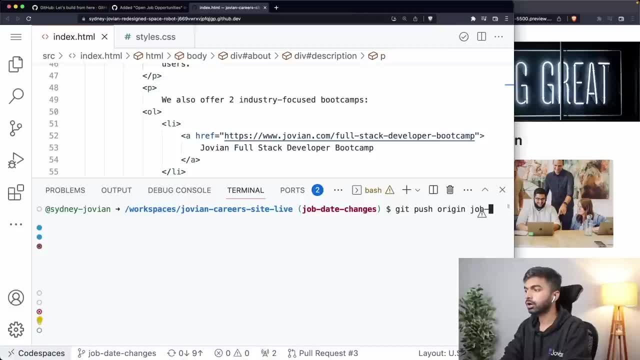 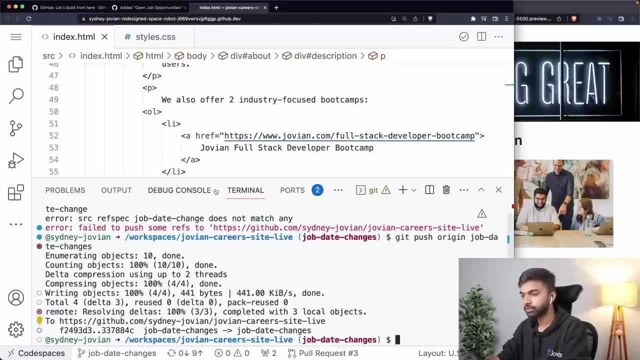 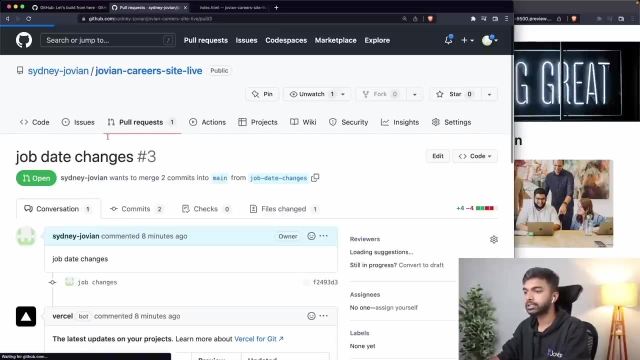 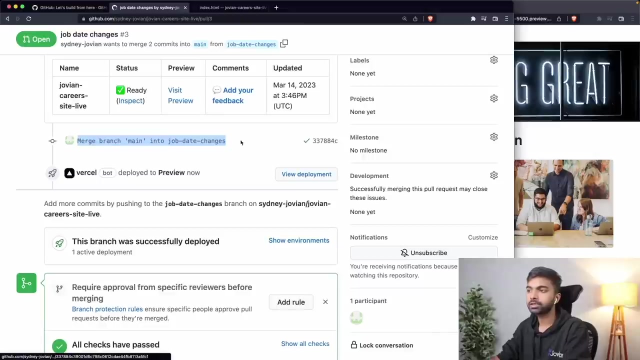 So get push origin job hyphen, date hyphen, change changes and this should get pushed. Okay, Finally, now we can come back here and we can see that job date changes has now been updated. Job date changes has now been updated with the merged changes into the main branch. 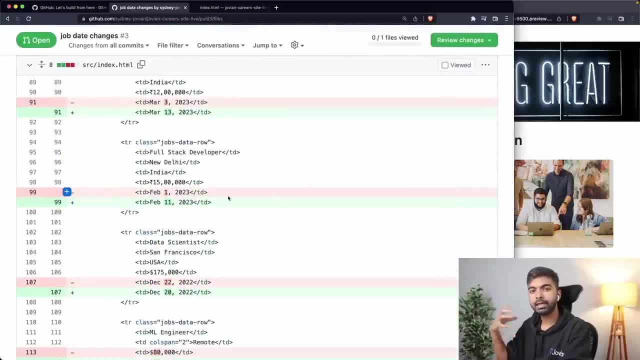 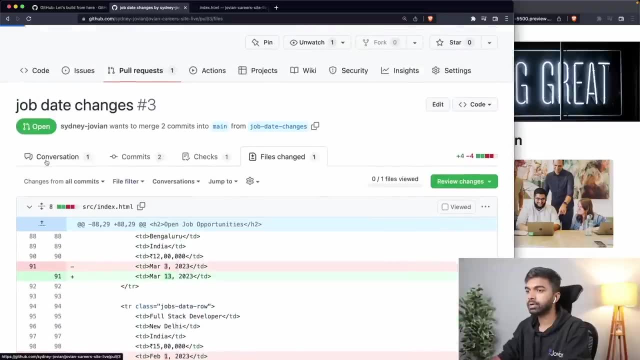 Okay, Okay, Okay, Okay. So this is the main branch that is present, And now somebody can come in and somebody can approve it, And then this can be merged in. Now we can go in and now we can merge this change and put that back. 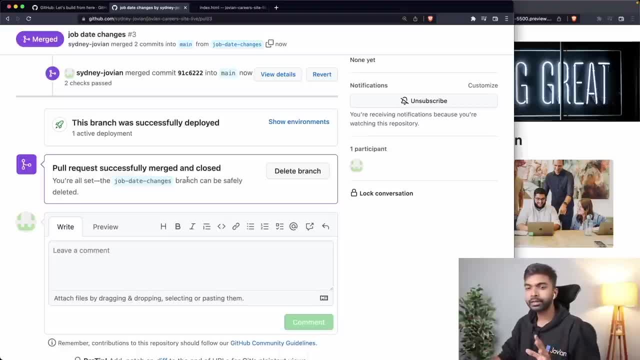 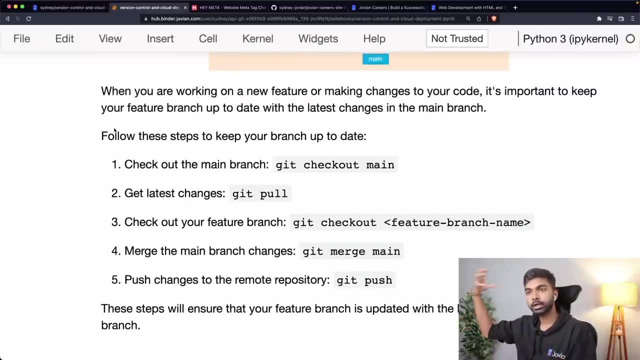 Okay, So I know that there was a lot going on there, but I'll just first revise this. So what we do is whenever new changes have come onto the main branch on GitHub and we want to incorporate them into our feature branches. Here's what we need to do. 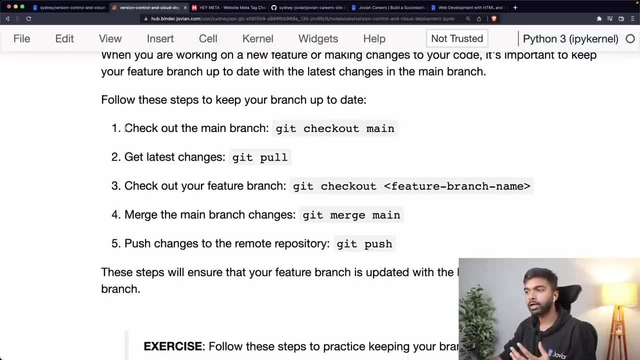 First We go to our code space or wherever we are We are doing our development. first go to the main branch, our local main branch, using get checkout mean. then we get the latest changes from the remote by by running get pull or get pull origin main, so that our local main is tracking at the same place where our 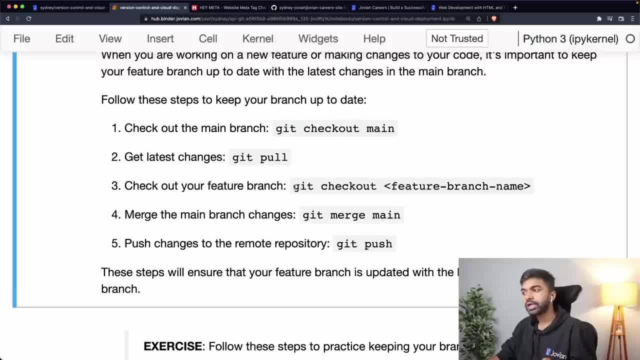 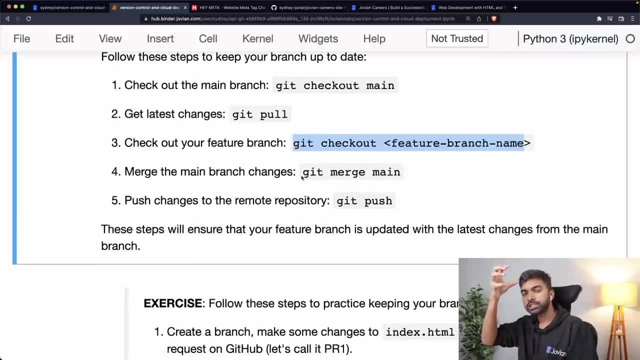 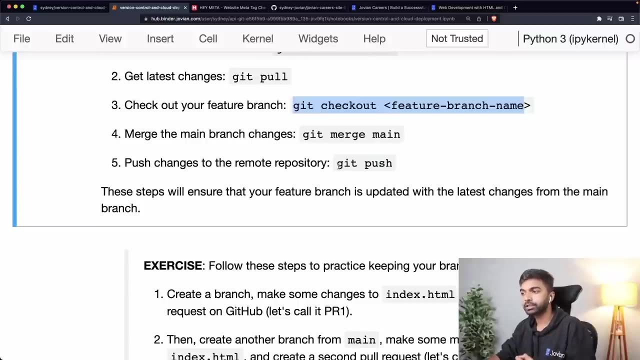 latest changes are on GitHub. Then we check out our feature branch. We say get checkout feature branch name. Then We merge in the changes from the main branch that we have locally now into our feature branch And finally we push these changes to the remote repository. 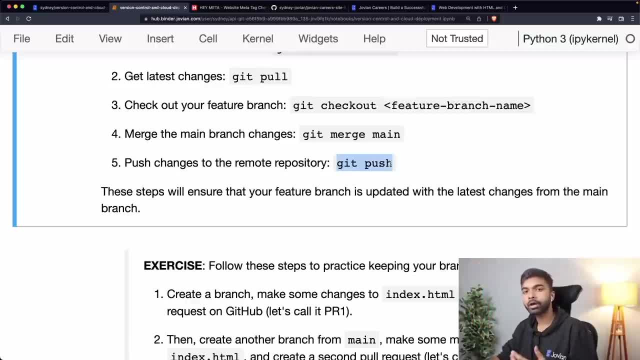 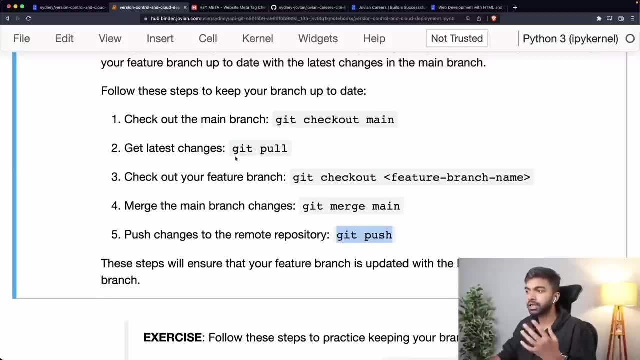 So we take our feature branch and push it to remote so that the pull request gets updated. Okay, So this is the workflow that you will do over and over as a developer: you'll check out the main branch, get pull, check out the feature branch, merge the changes from the main branch. 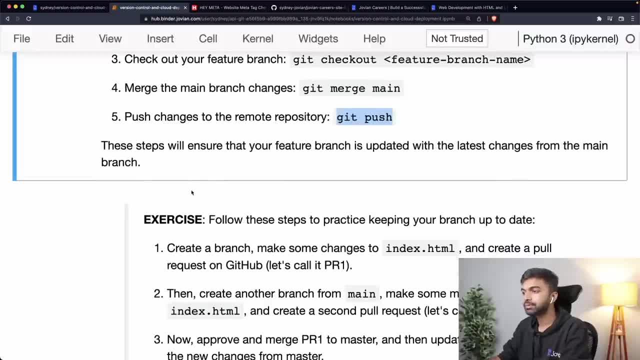 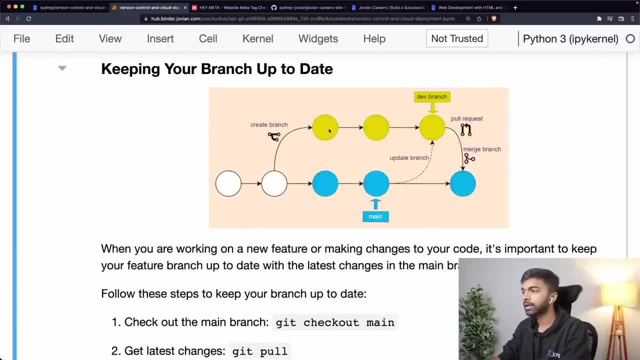 and then push your feature branch back to GitHub. Okay, Okay. Okay, So the pull request from the main branch is updated with the latest changes from the main branch. Okay, So, as you have a created a feature branch and you made some comments on it and made a, 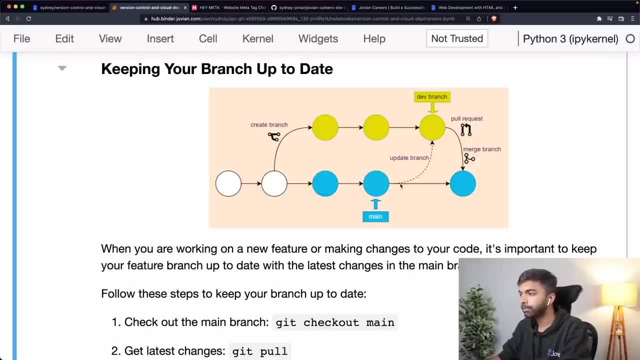 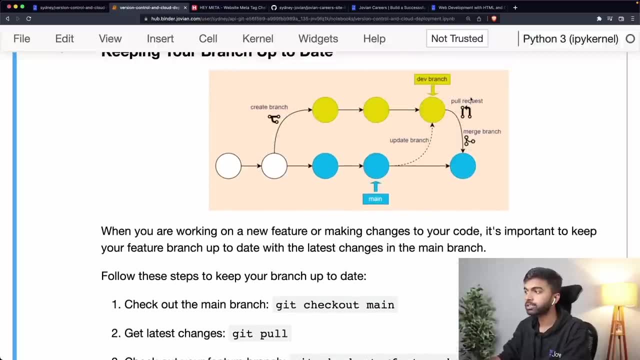 pull request. if new changes have come onto the main branch, you can simply pull those changes in by following this workflow, And then you can push your main branch back. push your feature branch back and your pull request will get updated, and then the merging will happen seamlessly. 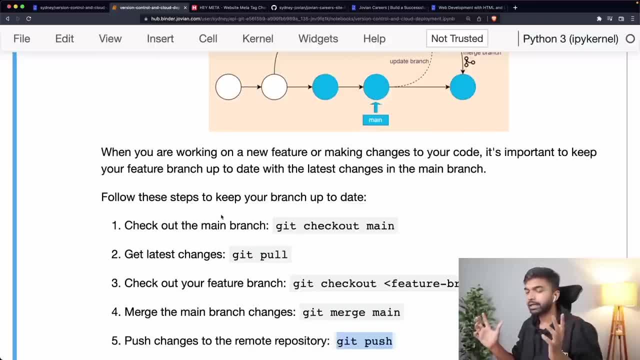 Okay, So that's how. that's how merging works. This is called Yeah, So you're basically merging changes from the main branch into the feature branch, And Git is smart enough that if the changes were made within the same file, but to different. 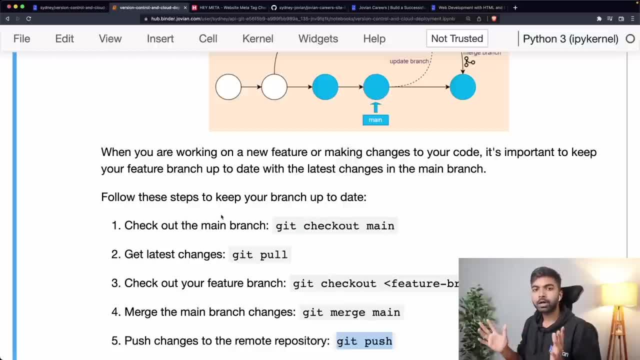 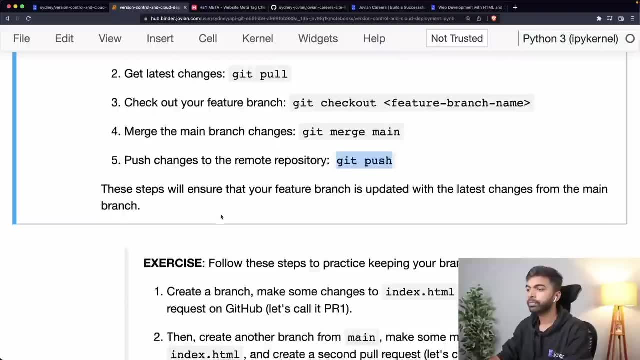 parts of the same file. then things will work out just fine. Git will be able to combine all those changes from multiple users, multiple commits, together. Okay, And again, I encourage you to practice this. create a branch, make some changes, create. 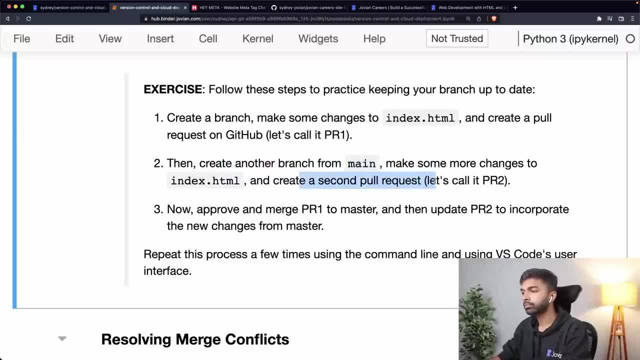 a pull request, create another branch and make some changes. create a second pull request Now. approve, approve and merge the first pull request- Okay- And then update the second pull request to incorporate the new changes from the first pull request and repeat that process a few times using the command line and using VS. 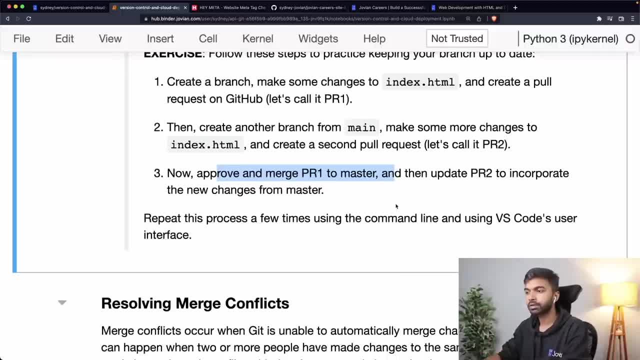 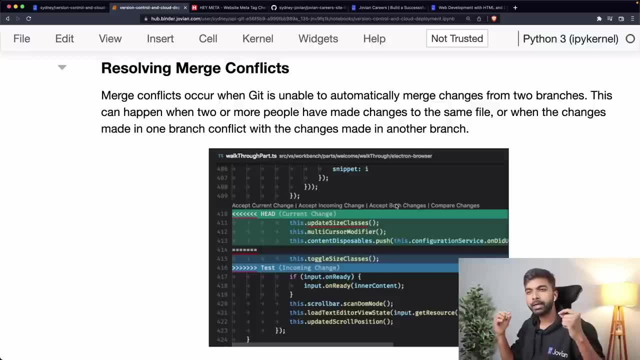 codes user interface to see if you understand how this whole thing works. Okay, Now there are certain cases where two people in two separate PRs have updated this exact same line of code, in which case there is going to be something called a merge conflict. 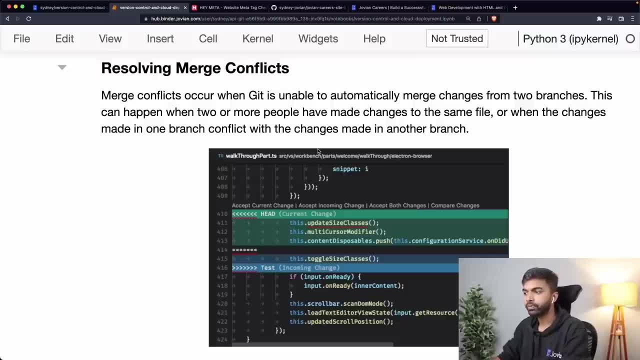 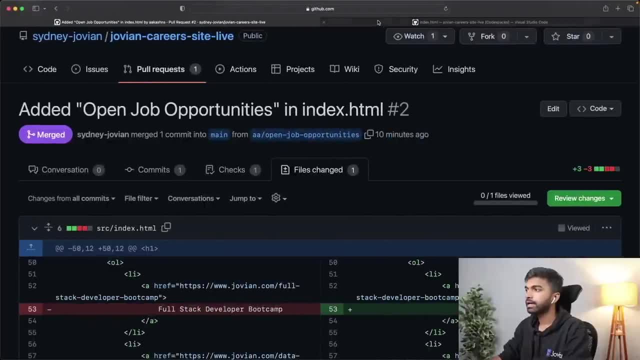 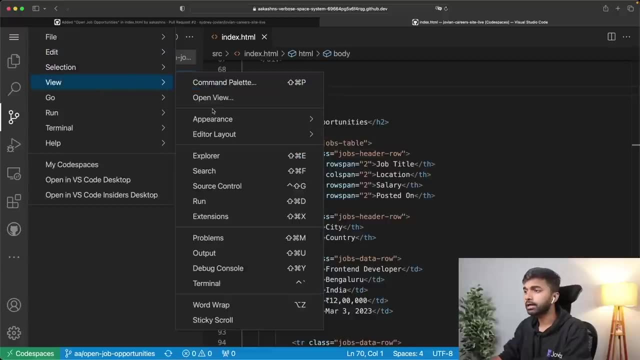 So let us try and simulate a merge conflict situation Now By both users updating just the title of the page. Okay, So let's do this. Let us first go back here into the code space that is being used by the user Akashns. 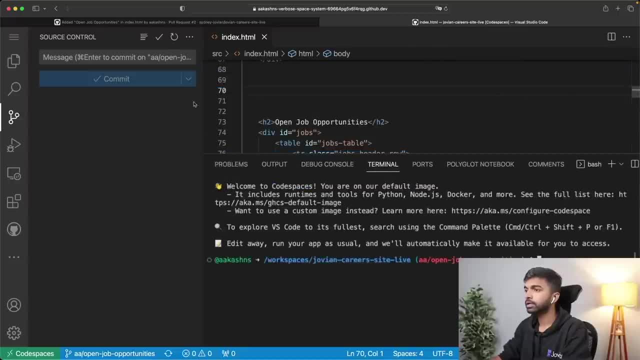 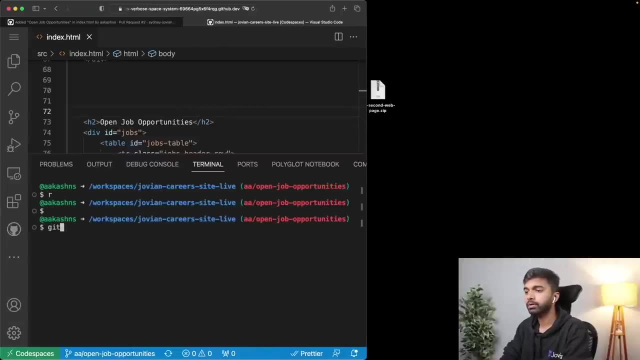 And let me open up a terminal. I'm just going to do everything on the terminal so that things are super clear. So we are currently on the branch open job opportunities. I'm going to first check out the branch- Git checkout main. Okay, now I'm on the main branch on my Akashns code space. 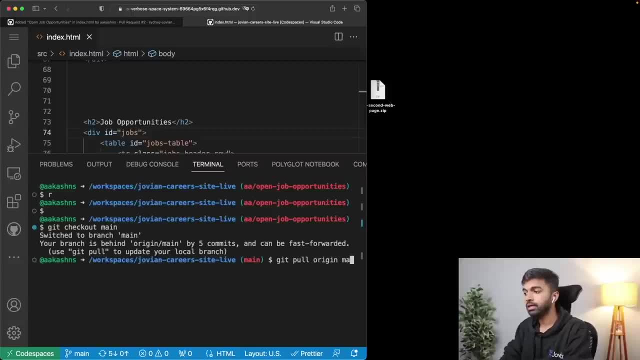 Then I'm going to run git pull origin main so that I have the latest changes. Perfect, I am going to get the latest changes on the Sydney account as well shortly, But now I'm going to create a new branch. I'm going to create a branch, git branch. 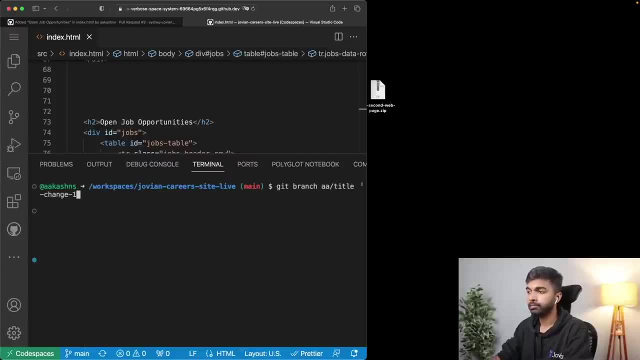 A hyphen. title change one. Okay, I've created a new branch. title change one. I'm going to check out that new branch. Git checkout AA. title change one. So now I've checked out a new branch, So I have the latest main branch from the latest main branch. 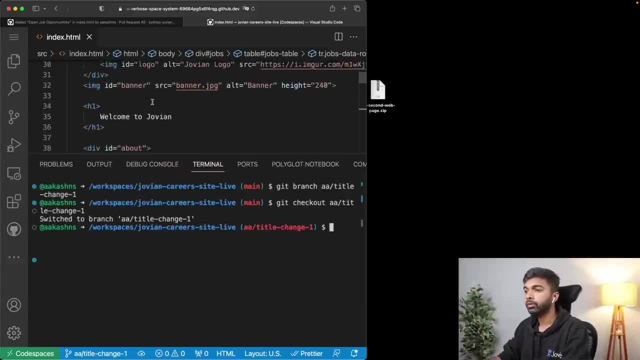 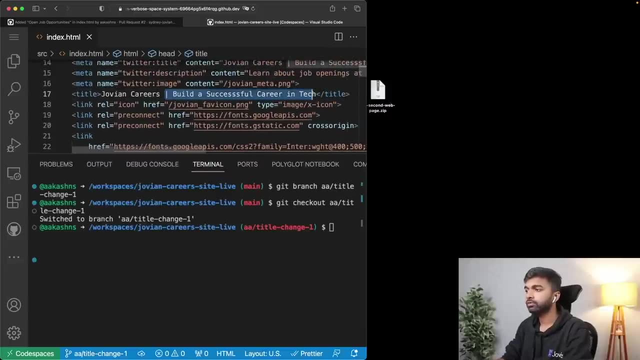 I've checked out a new branch. Now I'm going to come in here and I'm going to change the title of the page, which is: I'm just going to change it back to Jovian careers. Okay, So I'm changing the title of the page to Jovian careers. 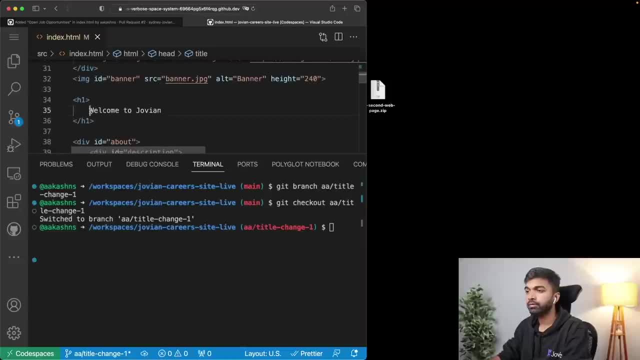 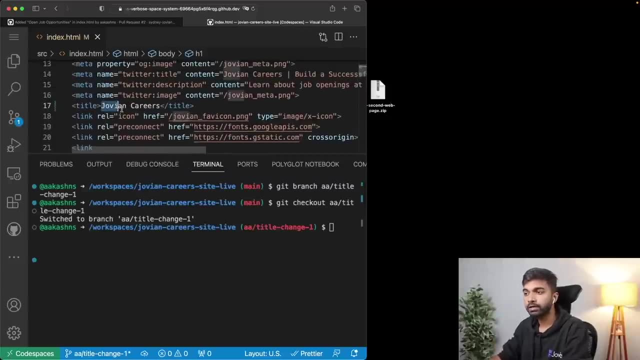 That is one change I'm making And I will also change your welcome to Jovian to about Jovian. So two changes I'm making. I've changed the title to Jovian careers and I have changed well, about Jovian to welcome to Jovian, to about Jovian. 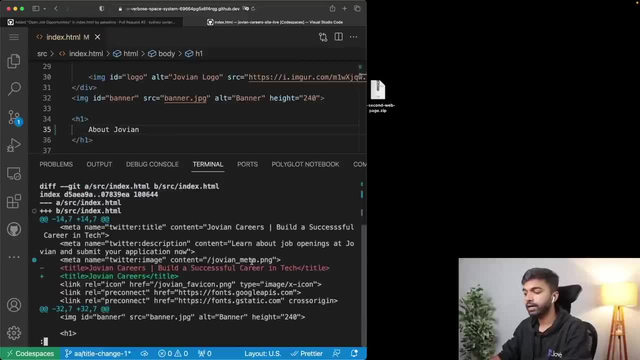 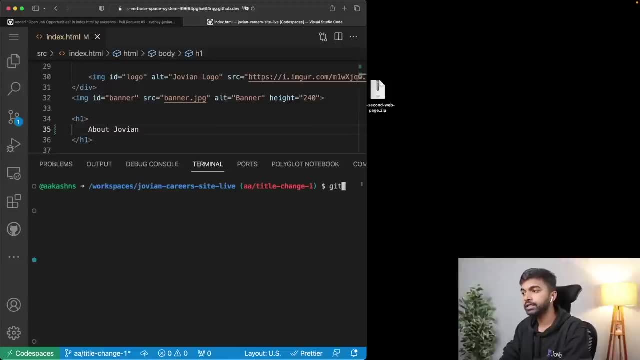 So those two changes, and you can verify these changes by using git diff. I can see that those are the only two changes I have made. Now I'm going to commit These changes. So I'm going to say get add dot and I'm going to get commit minus M. change title and. 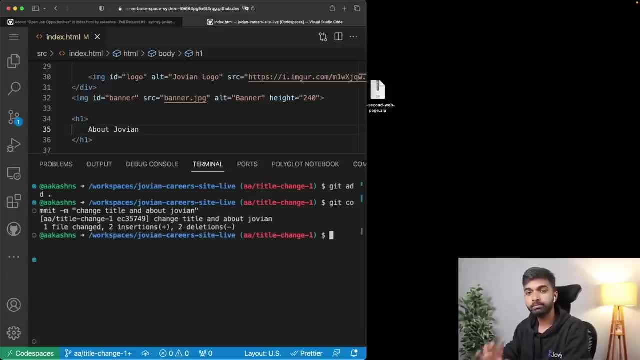 about Jovian. Okay, Now I have committed my changes onto my local branch and now I'm going to push my local branch to the to GitHub. but I'm going to say: get, push. origin AA hyphen. title change one. 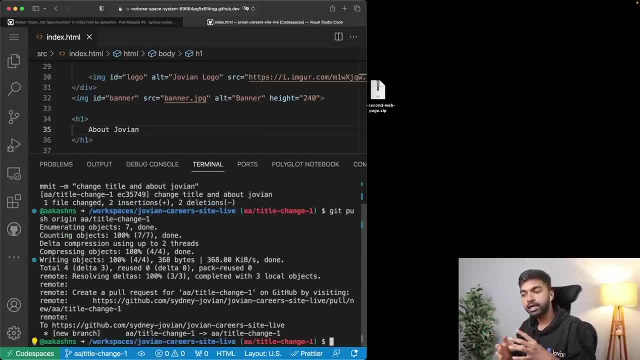 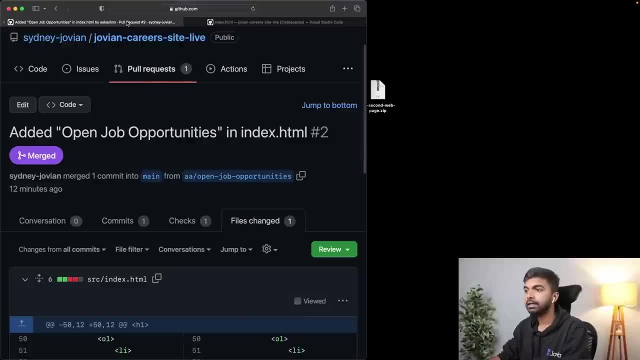 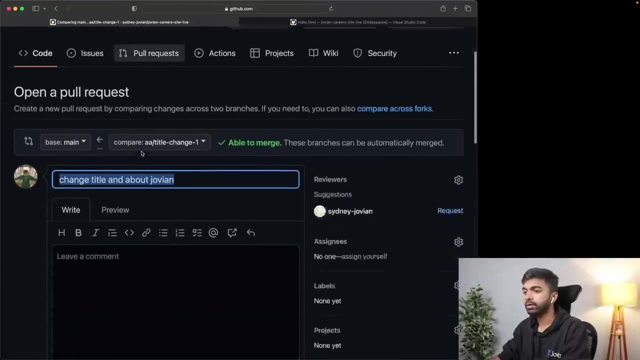 So now my branch, Which is based on the latest main and has a couple of changes- one to the title and one to about Jovian- has been pushed And now I can create a pull request using this branch. Okay, Now I can go in here and I can say create a pull request. 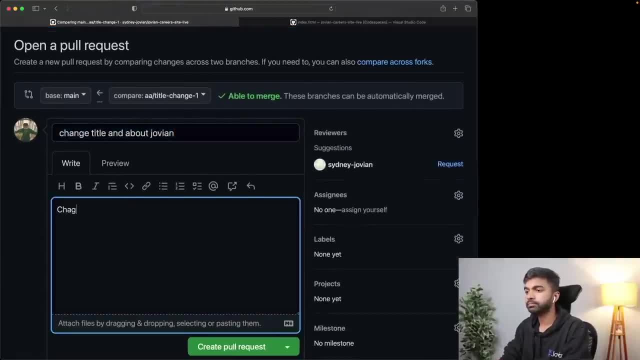 I'm going to just call it change title. So I've changed title to Jovian careers and then change Okay. Okay, So I've changed the description heading to about Jovian, Okay, And I'm going to create a pull request. 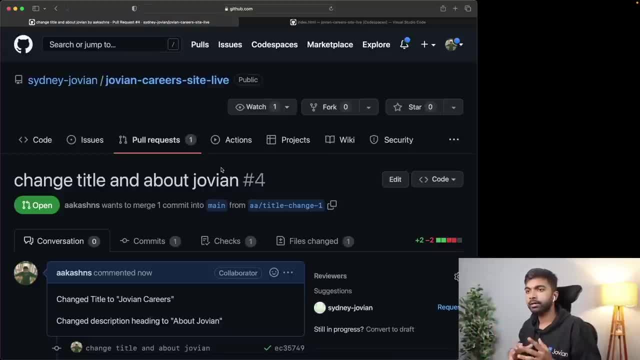 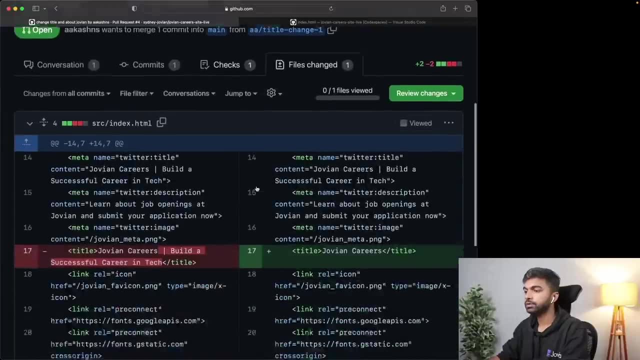 Perfect. So we understand this flow so far. we created a branch, We made some changes, We committed and we pushed. it created a pull request and we can verify that it contains only these two changes. It contains a change- Jovian careers- and it contains a change about Jovian. 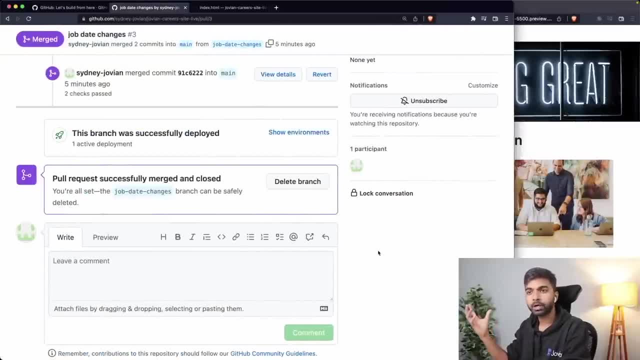 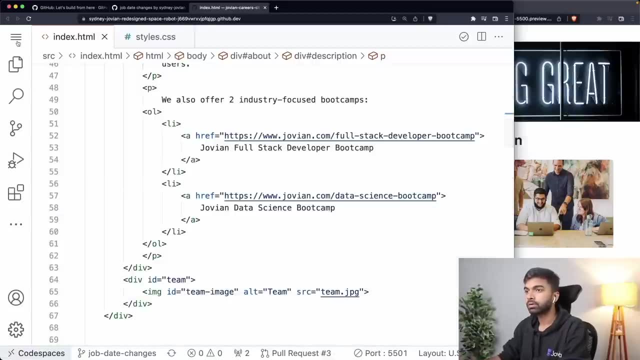 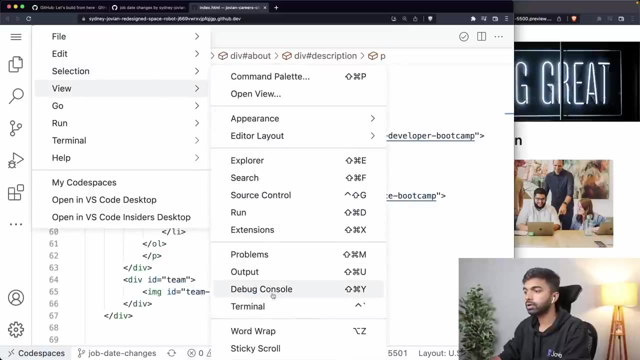 Perfect. Now, let's say, before this pull request was merged, Sydney was also working on some changes where he's going to change the title. So I'm going to save file. view terminal, or sorry, view terminal. I'm opening up the terminal again. 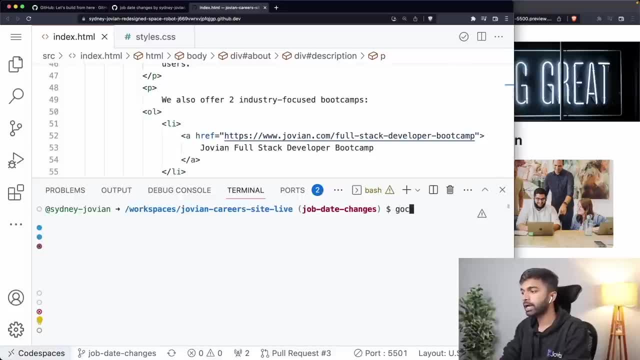 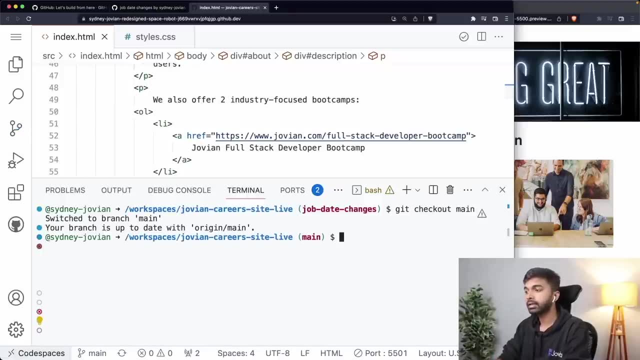 Let me reset it. Let me also go back here to the master. So let me say get checkout mall, or let me say get checkout main. So now I'm on the main branch back, Let me also do get full origin main. 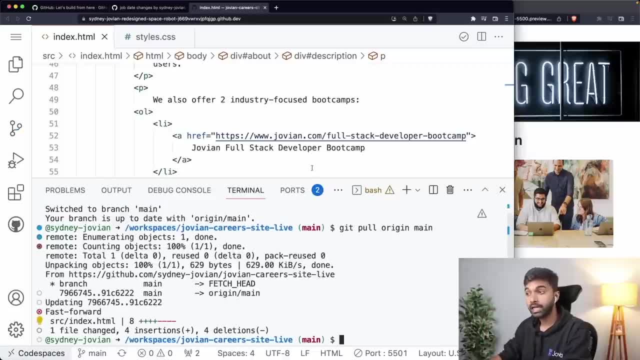 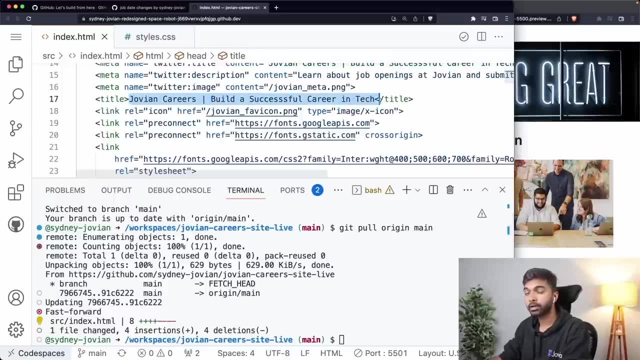 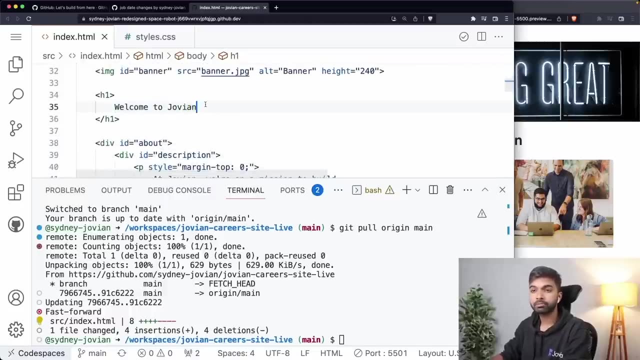 Okay, This is the latest version of the origin main. Okay, So in the latest main our title still has Jovian careers- build a successful career in tech, and the title here for the description is still welcome to Jovian because the changes. 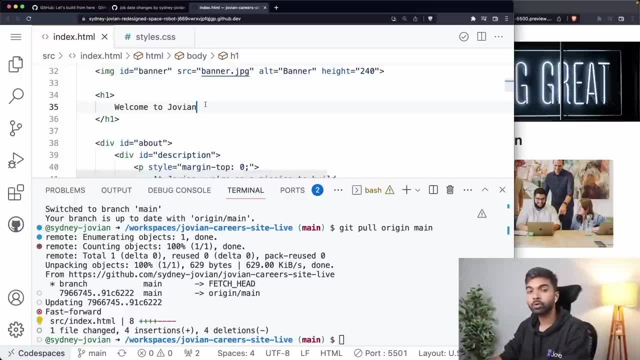 were made in a pull request that is not yet merged to main. Okay, So I hope this is clear to you- that our main branch is still still has the old title and the old heading. Okay, Now I'm going to create a new feature branch. 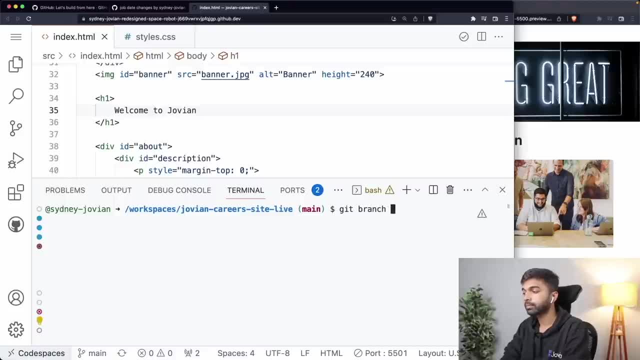 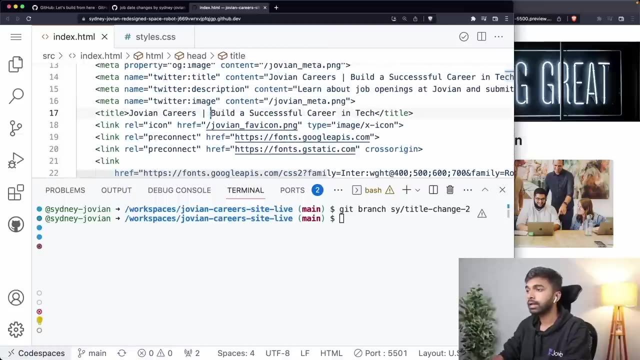 So I'm going to say get branch SY for Sydney title change to okay, fine. And now I am going to come in here and I'm going to remove this part, Okay. So I'm just going to remove the part. build a successful career in tech. 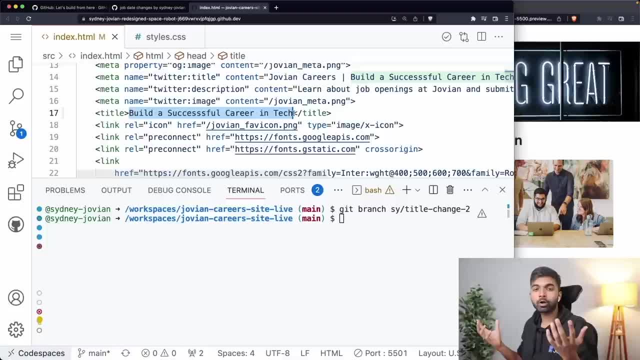 I'm going to keep the part: build a successful career in tech. So maybe two people got different instructions. Akash has made the change to about Jovian. He was asked to shorten the title and Sydney also got the instruction to shorten the title. 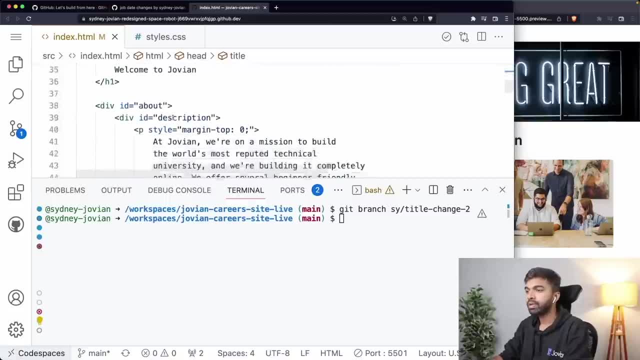 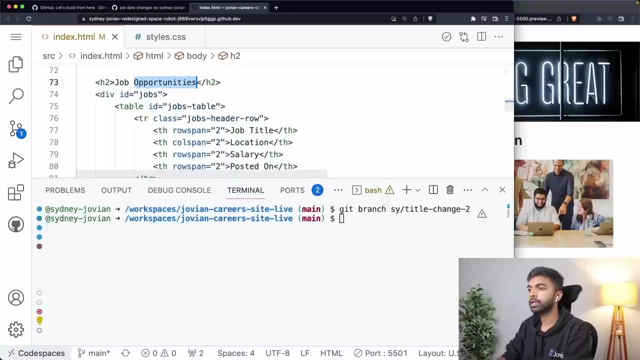 and he changed it to build a successful career in tech. And maybe I also go in here and change something about the job opportunity. So I don't want it to say open job opportunities, I want it to say job openings- Okay, And I have, I will also check out this branch, get checkout SY. slash title, change to and. 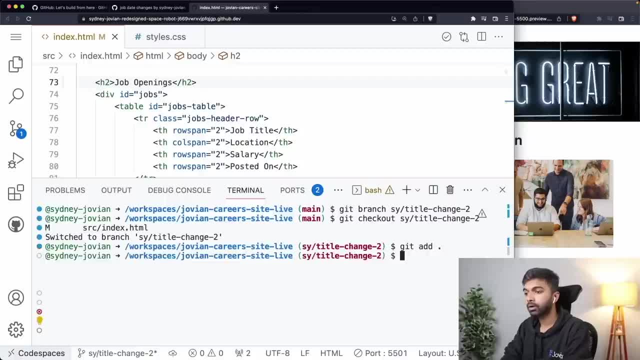 once I've checked out the branch, I'm going to add the changes. So get add dot. then I'm going to say, get commit minus M, change title and job opportunities. Okay, Now I've committed, Now I'm going to push this branch. 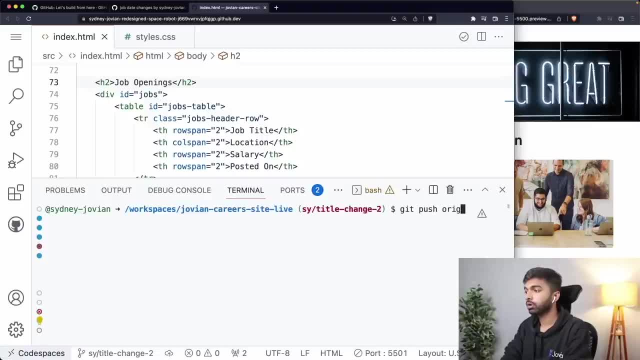 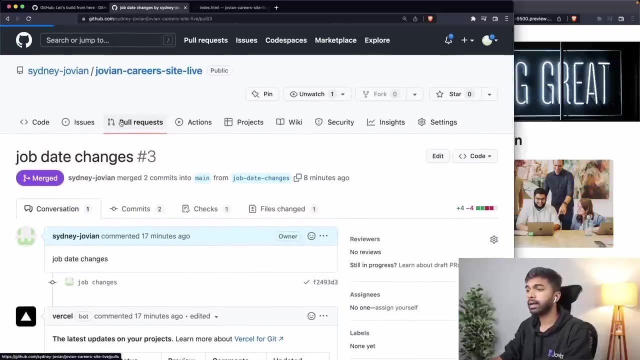 So I'm going to say: get push, origin SY slash title change to: Now my branch has been pushed to the origin, which is GitHub. Now we can come back here and create a pull request, And here I am changing the title. 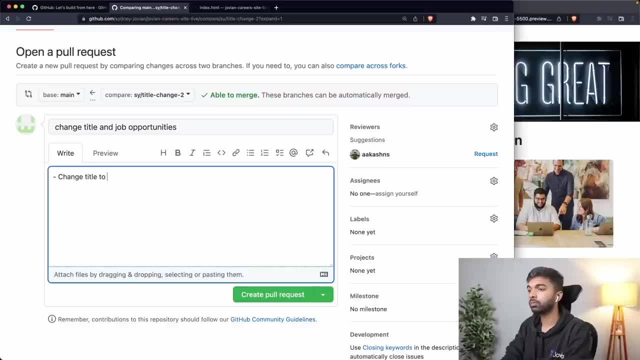 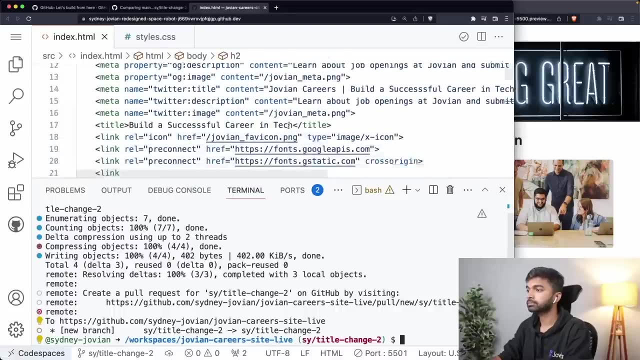 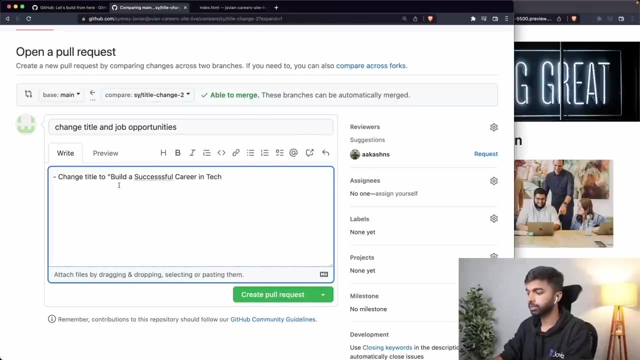 So change title and job opportunity. So here I'm changing the title to build a successful career in tech, Right, Yeah, So the title is changed to build a successful career. So I'm going to say business in tech and then the is the job section. header to job. 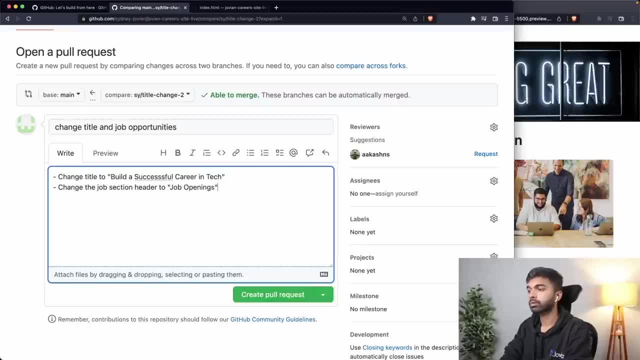 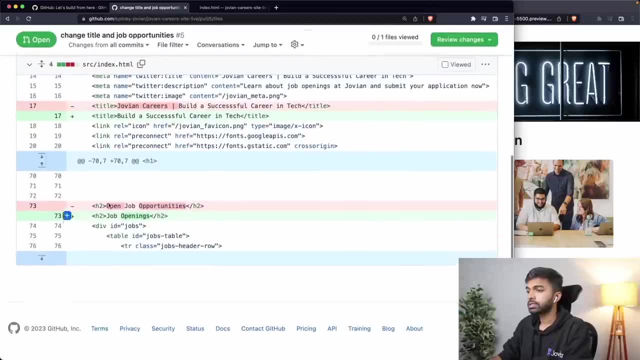 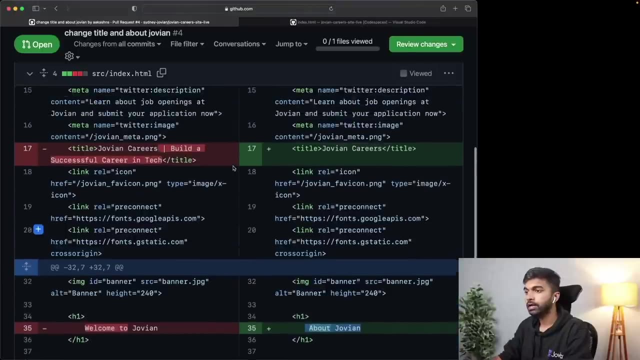 openings. Okay, Let me create a pull request here and let's see now. So here now there are two changes on the title and on job openings. You're also. there are two changes on the title, but a different change to the title. 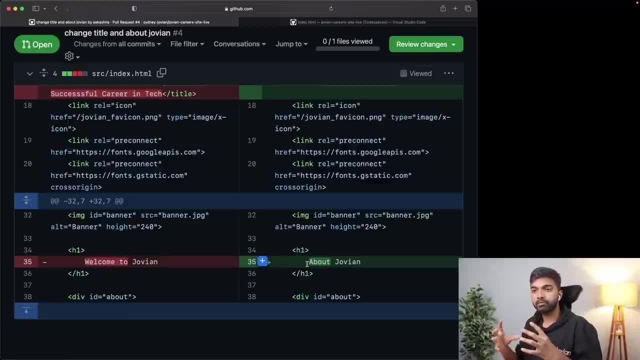 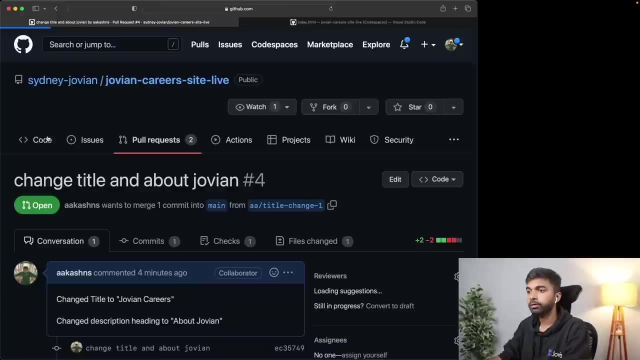 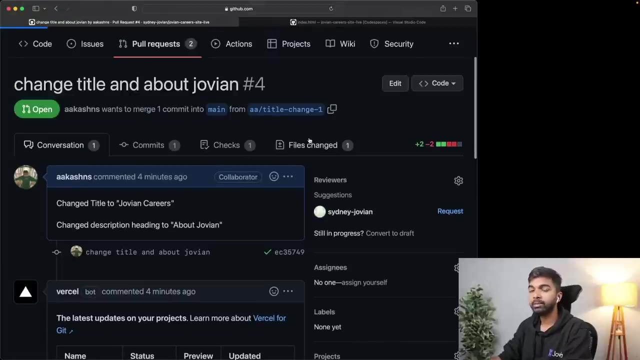 and on the job openings. Okay, These are made against the latest version of master. Now let us merge one of the pull requests. So now let us go in here and let us merge this first pull request. So what will happen is that when, by merging this pull request which changes the title, 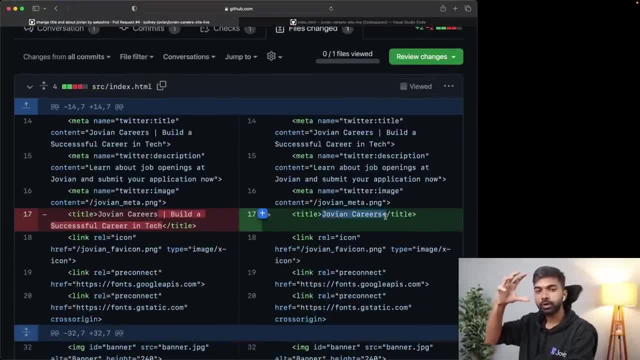 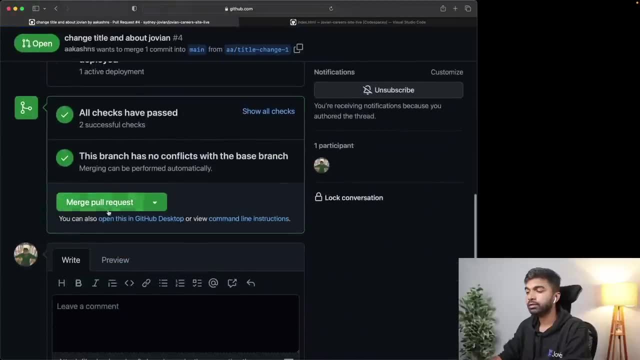 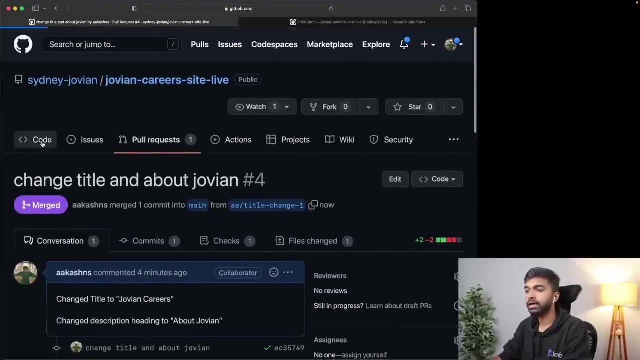 to Jovian careers in our main branch. we are going to get back Jovian careers as the title. Okay, So I'm going to go in here and I'm going to check more. Click merge. pull request confirm merge And the pull request has been merged and I can verify if I go into code and check the. 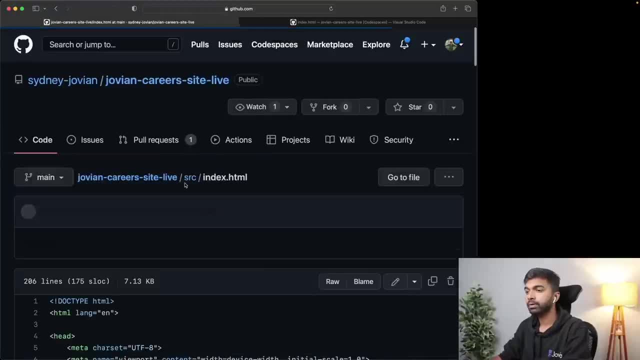 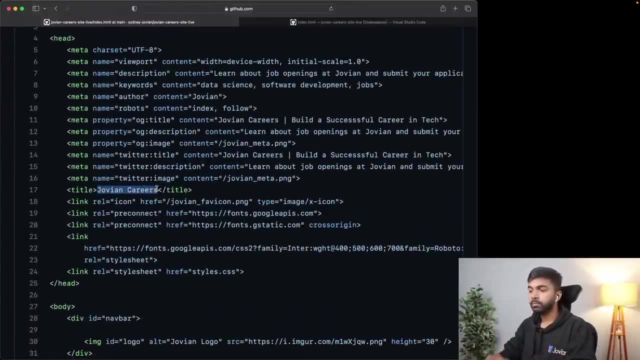 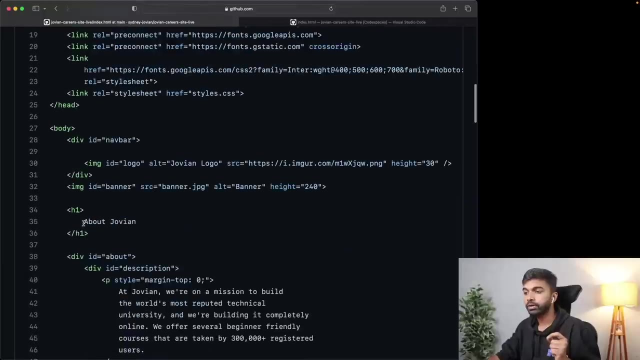 main branch and check index dot HTML. it is going to have the change title: Jovian careers. Okay, So now the first pull request has been merged, The title of the page has changed to Jovian careers and the header of the first section. 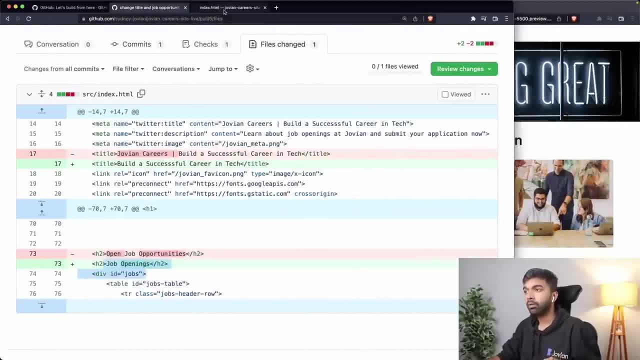 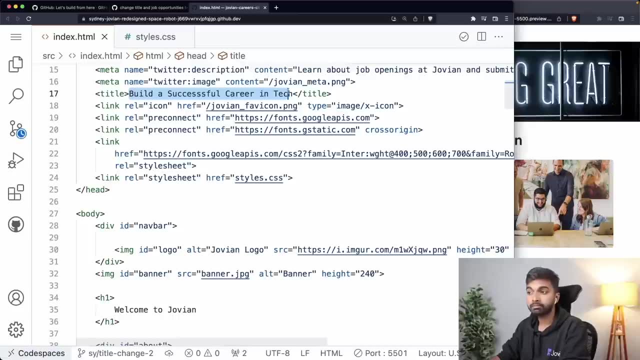 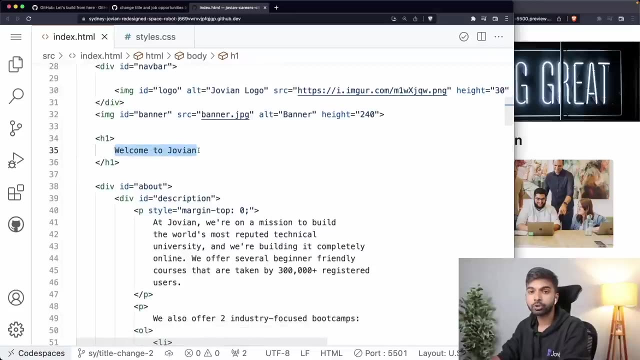 has changed to about Jovian. However, obviously for Sydney, the title of the change, the title of the page, is whatever they have set in their feature branch And the heading of the first section is welcome to Jovian and not about Jovian. 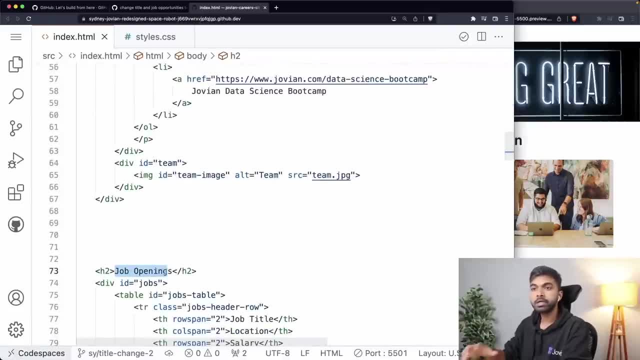 And of course, they've also made an additional change called job openings. So now Sydney's feature branch is behind the main branch on GitHub. So Sydney needs to update their feature branch. So let's update the feature Branch step-by-step. So I'm going to open the terminal again. 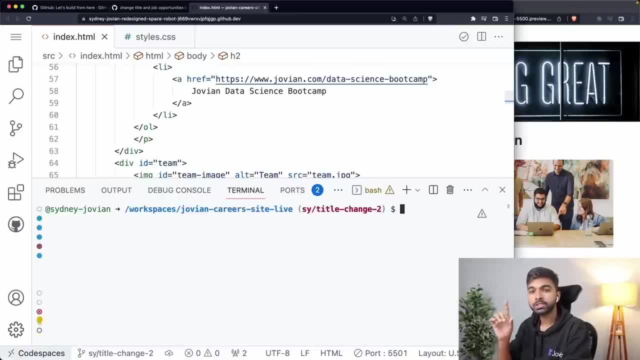 I'm going to reset things and remember the step-by-step process for updating the feature branch. First you go to get checkout main. first you get to the main branch, because our local main branch and code spaces is behind the main branch on origin. 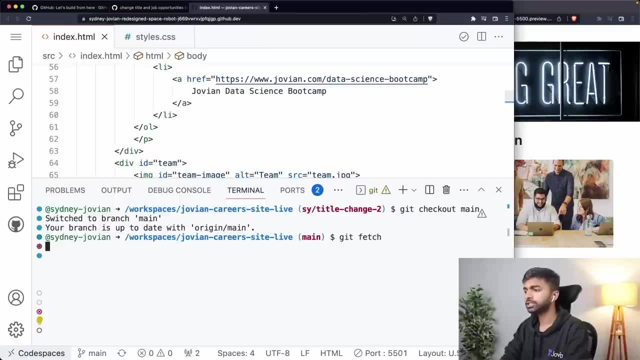 Then we can check using get fetch minus minus- all are just get fetch- how far behind we are. Okay, So we can say get status: Okay, So check that we are behind origin main. So we are behind the changes by two commits. So let us run git pull origin main. 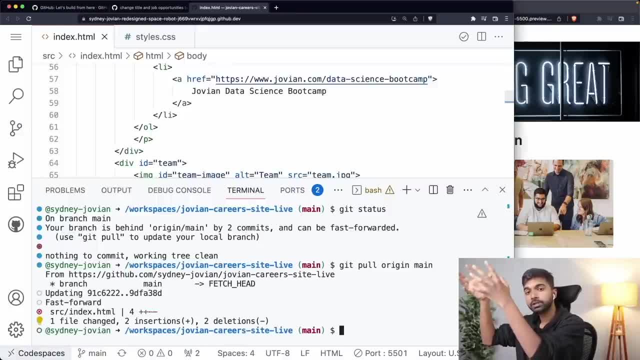 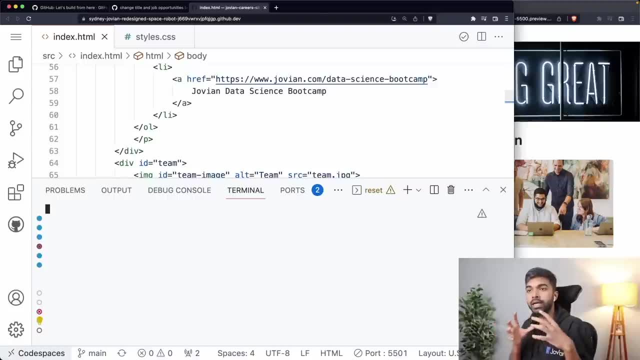 So now we are pulling the changes from the origin main branch on GitHub to our code space on the Sydney code space. Great, So now our main branch is up to date, but our feature branch is still tracking the old version of the main branch. 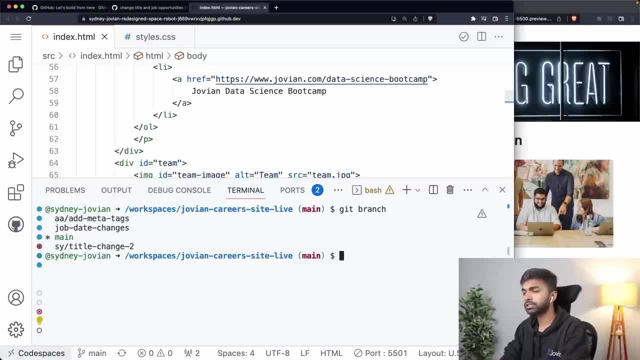 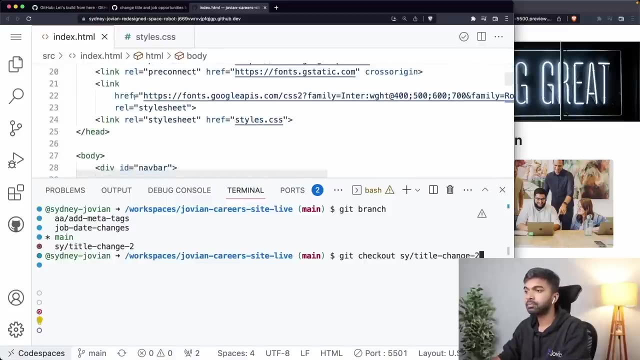 Now we go back to our feature branch. So let's check the name of the branch. Okay, The feature branches: SY title change to. so git checkout SY title change to: and, by the way, you can verify here that so far we are on the main branch and on the main branch. 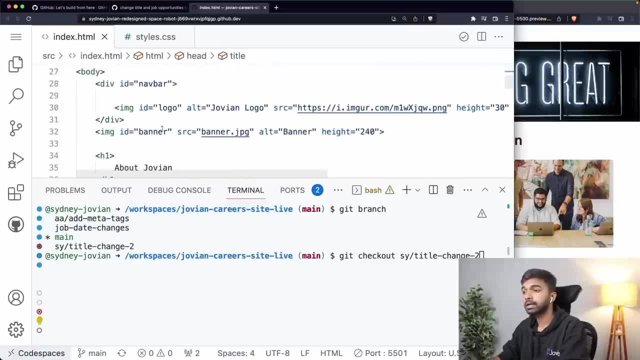 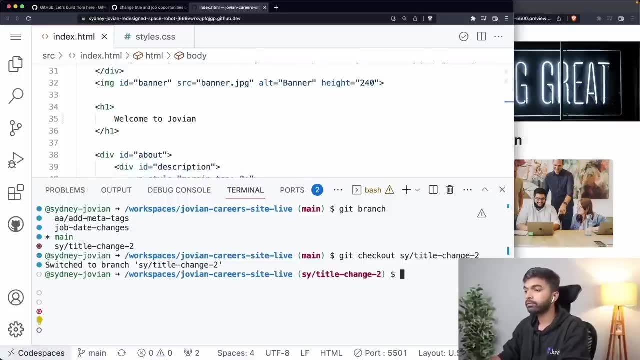 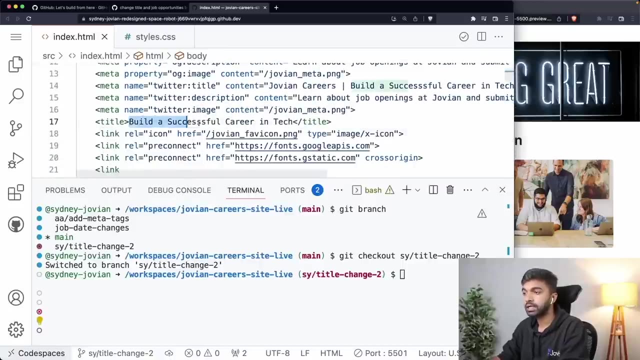 it says Jovian careers, which is the change that had been made by our caution is- and the title of the first section is about Jovian, which is also a change that was made by our customers. Okay, Okay, So now we have the title that was set by Sydney here. 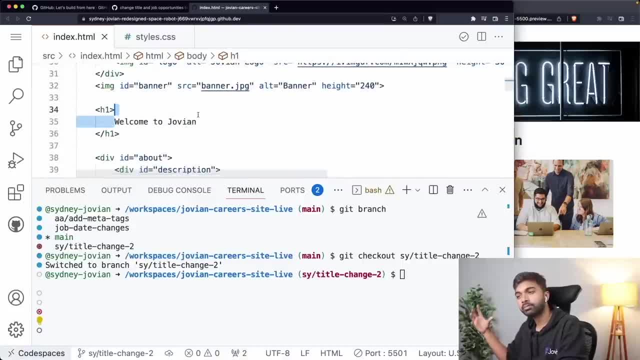 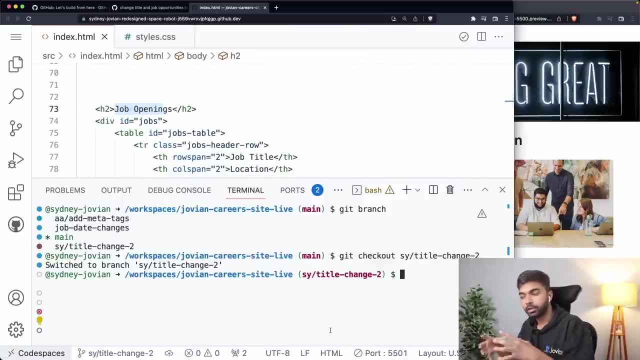 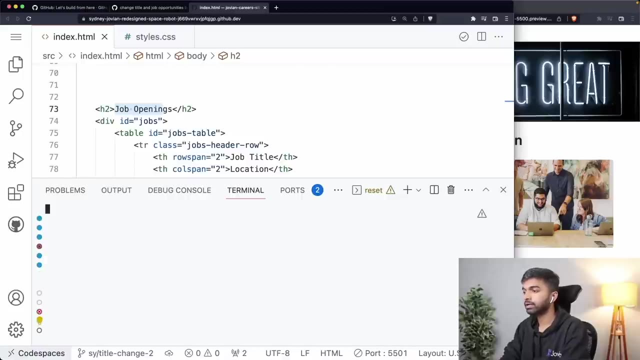 And now of course we have welcome to Jovian, because this is tracking the old main branch and we have this job openings here. Okay, So now we need to merge in the latest, the new main branch that we have just pulled in. So we say: git merge main. let me just reset that and type that again: git merge main. 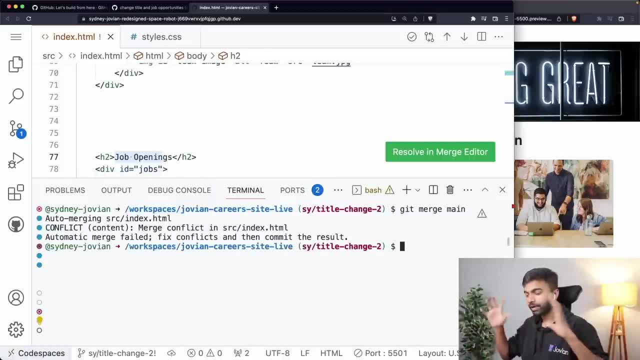 And here we are. Okay. So here is what happens. Okay, Finally, we've done all this set up to get to a point where, when I try to update my feature branch using the new changes that have come into the main branch, I run into 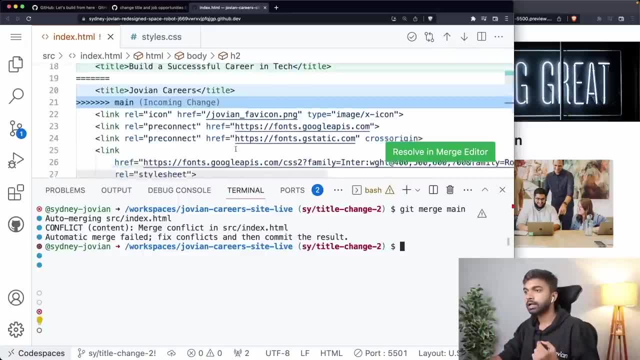 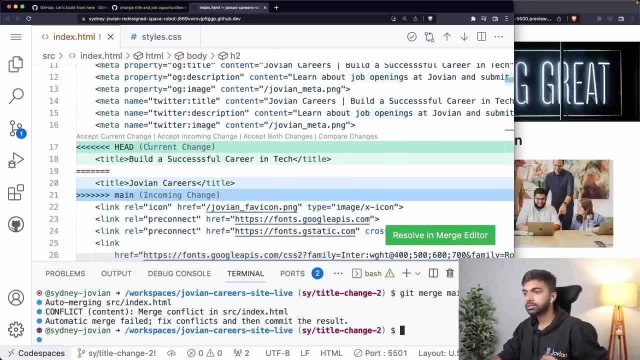 an issue because both of us are trying to update the same line. our caution is has updated, So there are two things. you have a current change, which is the change in my feature branch. So in my feature branch I have updated the title to build a service. 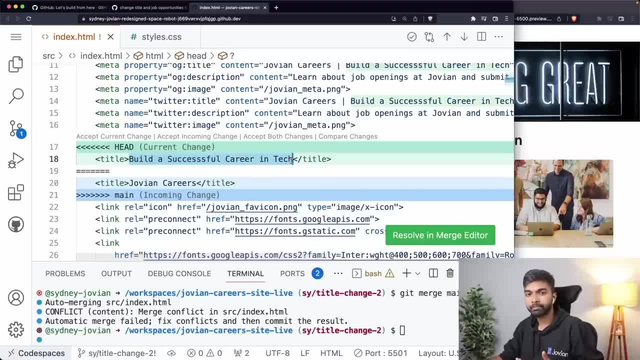 Okay, So build a successful career in Trek. However, when I try to merge in the main branch- the main branch that has come from GitHub- the latest main branch- because of some other pull request as the title Jovian careers- So both the main branch and my feature branch have been independently updated on this one. 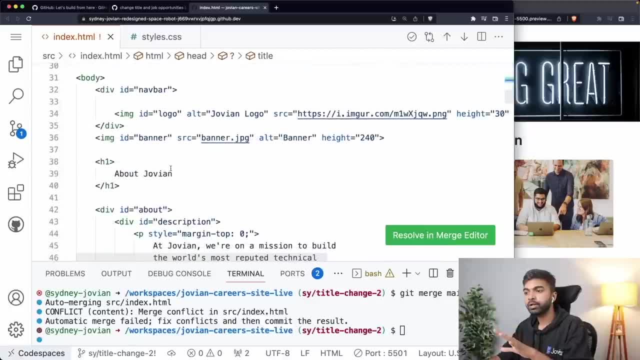 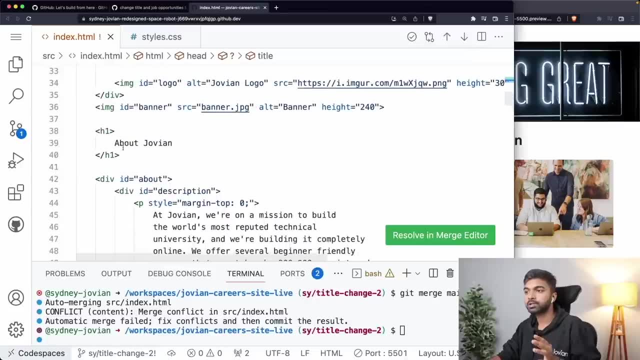 particular line And you can see only this. one particular line is an issue. This: this becomes about Jovian as expected- No issues here. And this becomes job openings- as expected- No, no issues here. Right, So this change came in from the main branch. 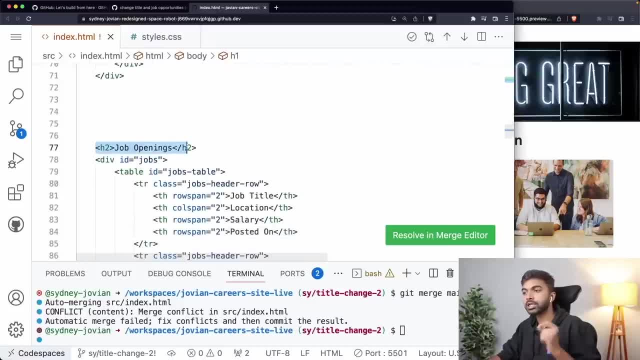 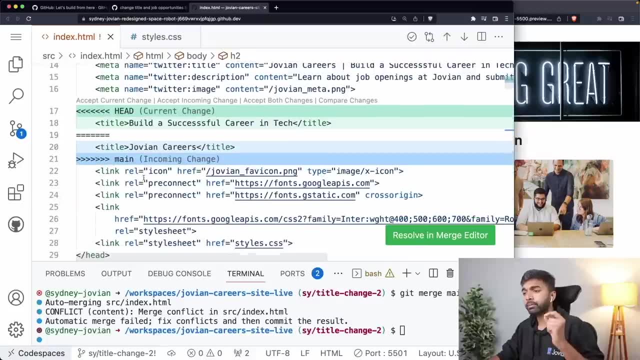 No problem. No, because we didn't change it in the feature branch. This change came in from the feature branch. No problem, because it was not previously changed in the main branch, but this change was made in the main branch as well, which is called Jovian careers. 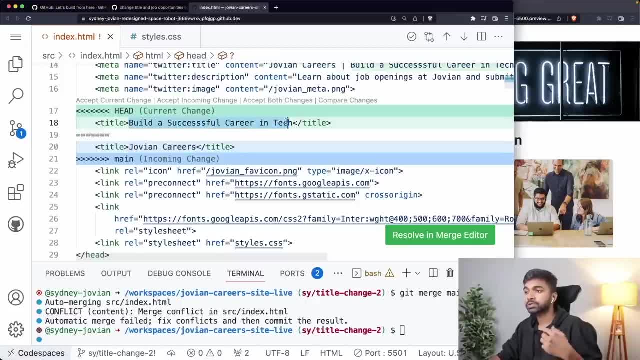 And this change was main made in the feature branch as well, which is called build a successful career in tech. So this is what Git does: It inserts this like random characters here, Which basically tell you that what you have on your current branch and what you have on 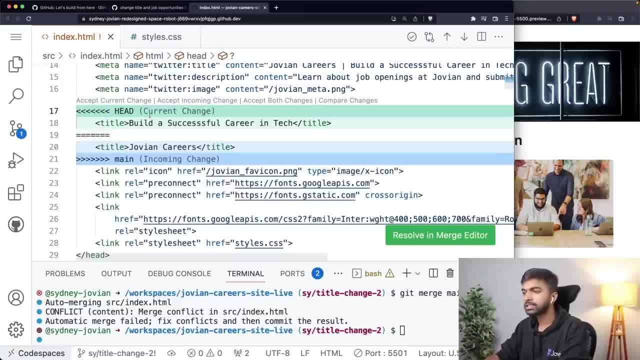 the main branch and you can either edit it manually- You can kind of erase all these characters- or you can just use one of these buttons- whether you want to accept the incoming change, which means the incoming changes, what is coming in from the branch you're trying to merge in, which is what is coming in for a 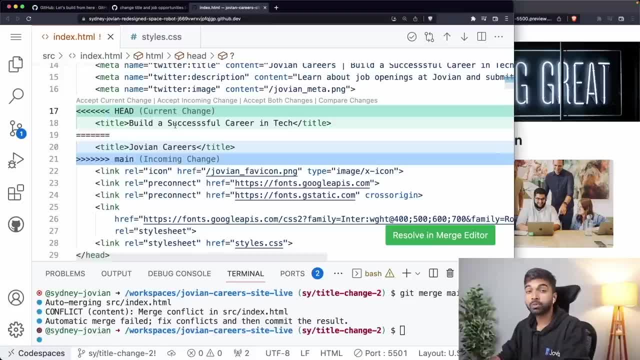 main. or you can accept the current change, which is what you have in your feature branch, or you can keep both changes. So here's what I'm going to do. I'm going to click accept current change. Okay, So I want my feature branch change to override what has come in from the updates in the main. 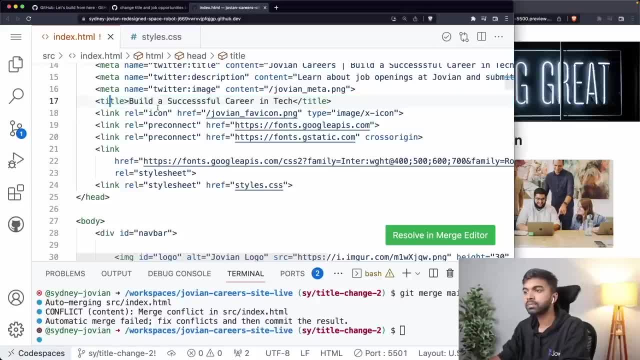 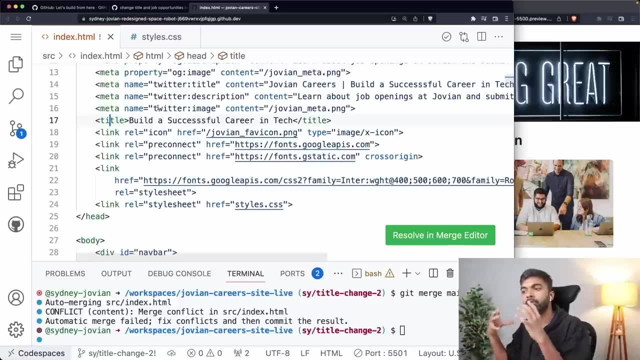 branch. So I'm going to click accept current change. And now in my feature branch I have overridden, I have resolved the merge conflict and I've overridden the change that was made in the main branch And now I need to create another commit. 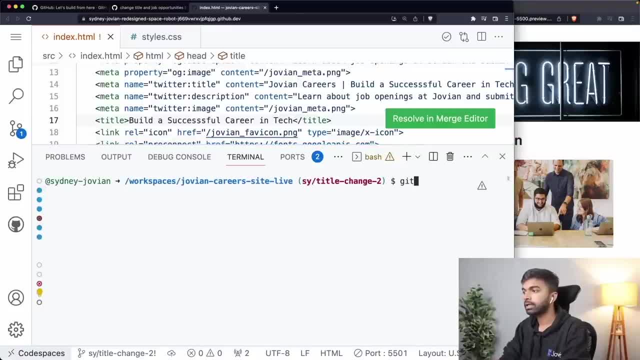 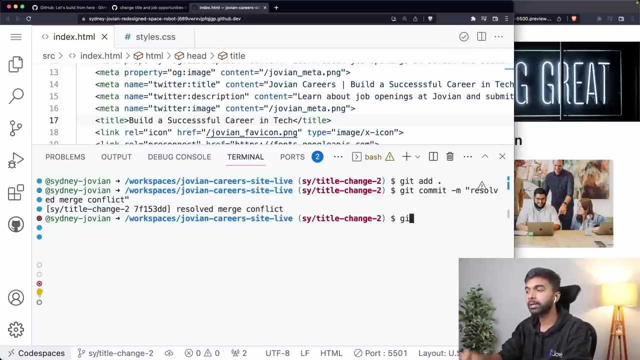 Okay. So now I can say: Git add dot. Git commit minus M. Resolved Merge Conflict. Okay, Now I've made this change. I need to push my feature branch to update my pull request. So now we can say: Git push origin SY title change to: okay. 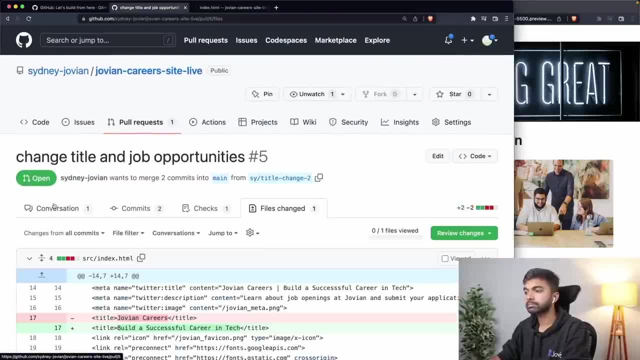 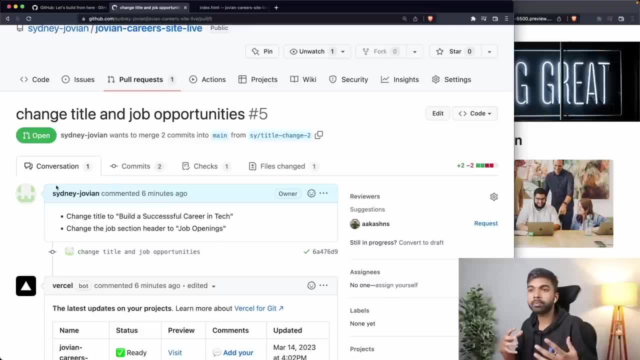 And now I can go back here and reload my pull request. So if I did not make this fix, this merge conflict and I tried to merge this pull request, it would say that The pull request cannot be merged because it is conflicting with the latest version. 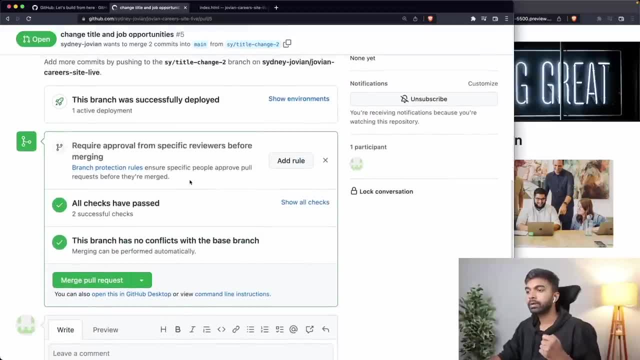 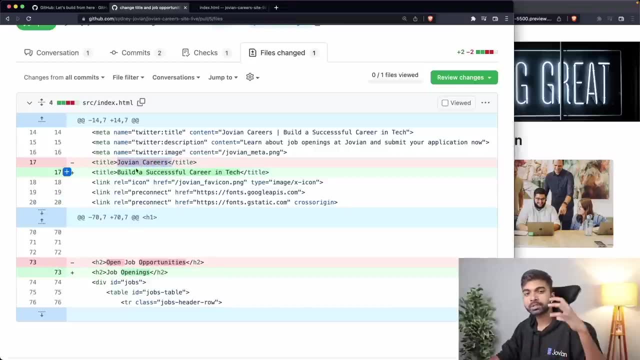 of main, But now that I've fixed this merge conflict, you can see that I have said that from the main branch. I want to change Jovian careers, which was the latest version of the title on the main branch, to build a successful career in tech. 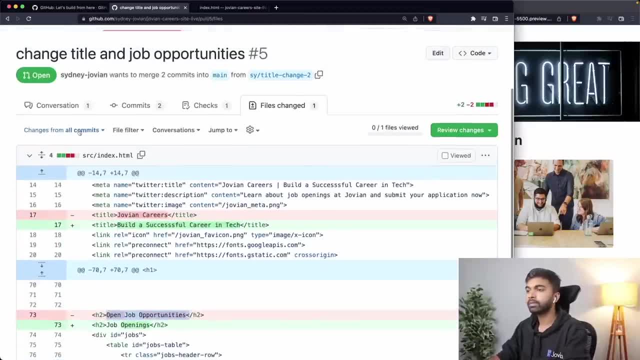 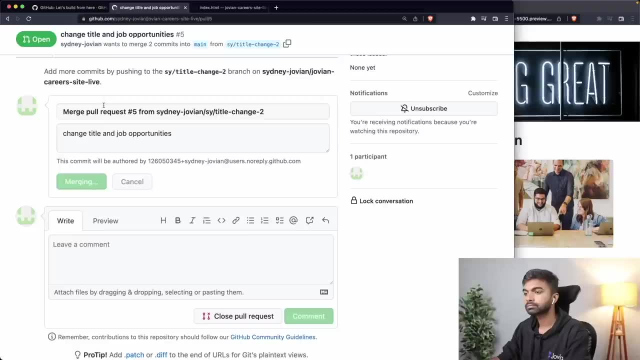 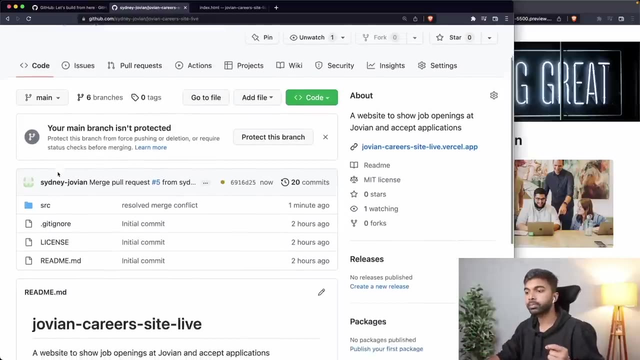 And I want to change open job opportunities to job openings. Okay, And then we can go ahead and merge this pull request. Right, And that's it. So now we should. on the main branch, we should have incorporated changes from both the places. 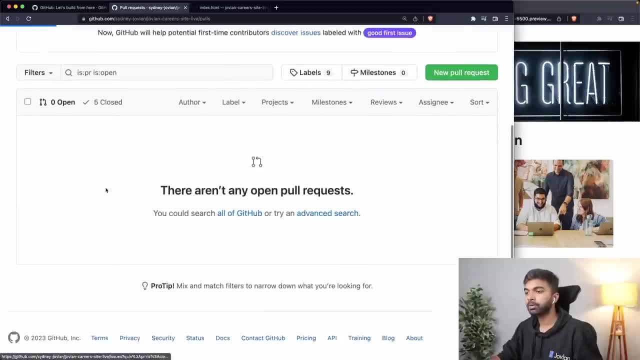 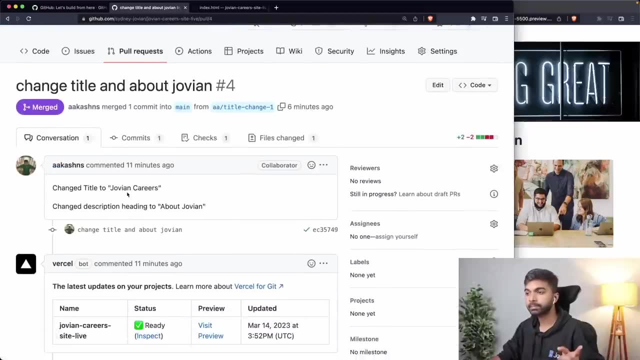 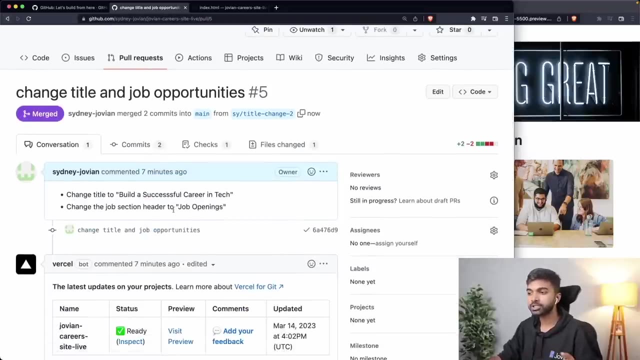 Right. So if we look back at the pull requests, we have closed a couple of pull requests. One of them changed the title to Jovian careers and about Jovian, which merged first. The second one changed the title to build a successful career and change the job section. 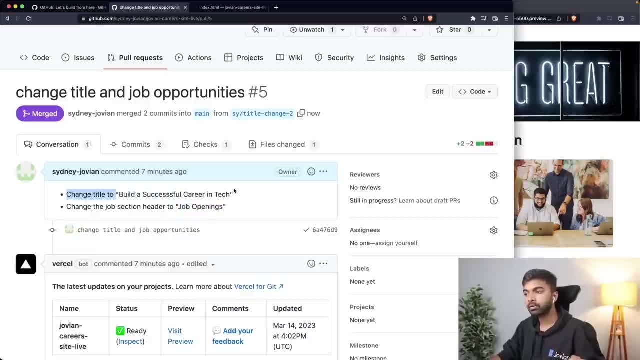 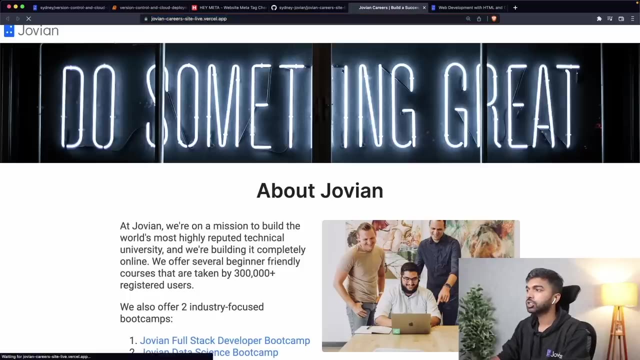 header to job openings, which merged second, And while merging the second one, Okay To override the changes from the first one. we could also have chosen to keep it. at the point of the merge conflict We can decide what to keep. So the end outcome of all of this is going to be that, if we just check the title here, 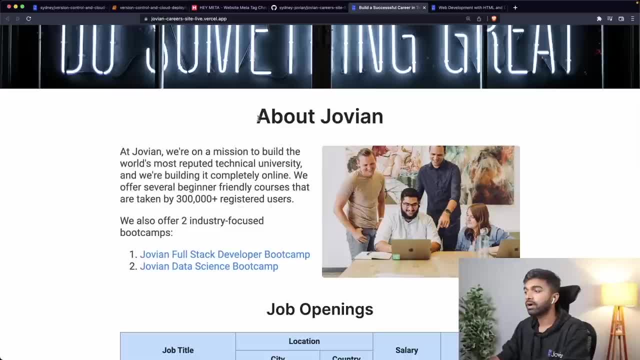 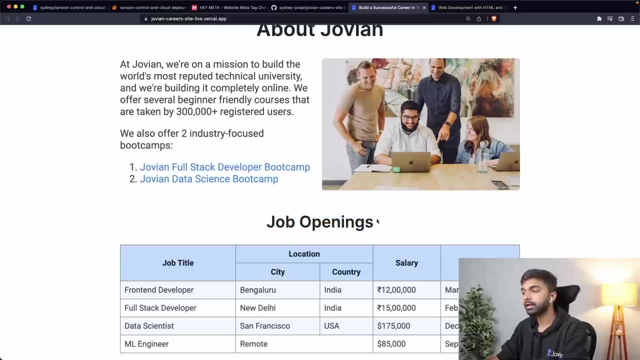 so the title becomes: build a successful career in tech. We have about Jovian. This came from PR, one from the PR by. our caution is: we have job openings. This came from PR to the PR created by Sydney Jovian. and this is how you reconcile changes. 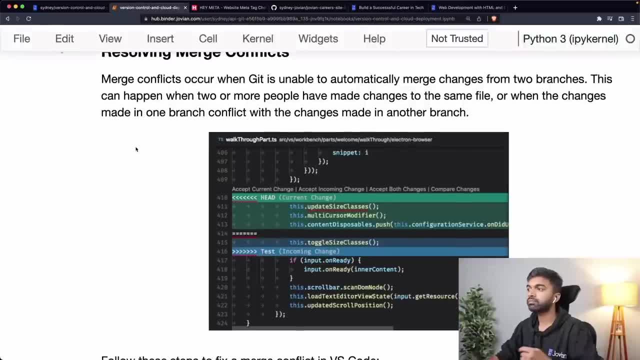 Okay, So just to recap how you resolve a merge. conflicts occur when Git is unable to automatically merge changes from two branches, And this can happen when two or more people have made changes to the same file or the same line in of code in a file. 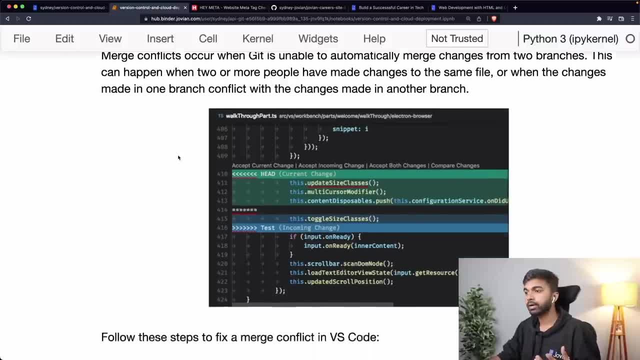 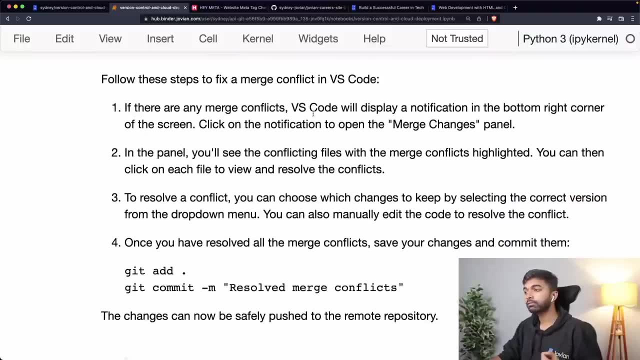 And the changes made in one branch conflict with the changes made in another branch. Okay, So these are the steps to build a fill, fix a merge conflict. So when there is a merge conflict, VS code will display a notification in the bottom right corner. 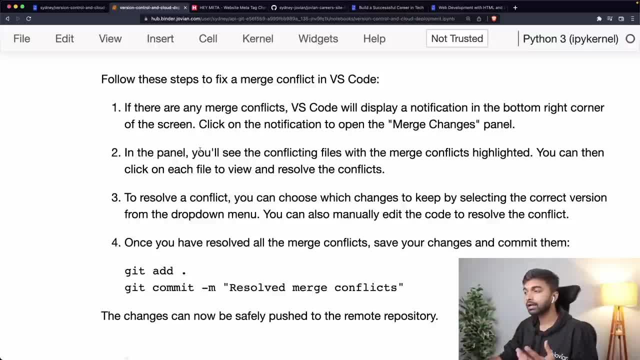 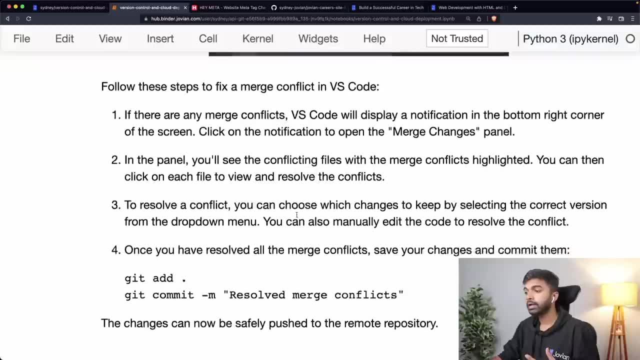 It will also show a way to merge changes. there You can see the conflicting files. so you can see it like this and you can have multiple files. You can have multiple conflicts within a single file And then for each file you can choose with changes to keep and how to select and select. 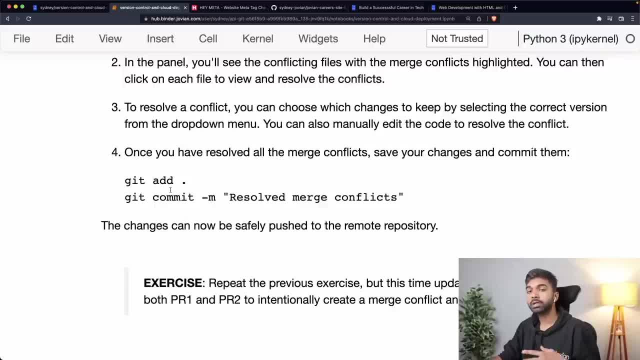 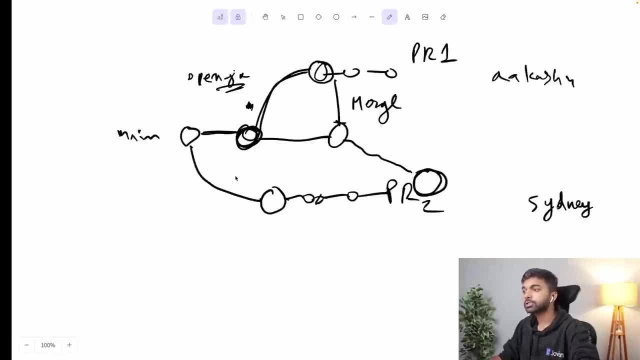 the right version, And once you have resolved all the merge conflicts, you need to make a new commit And then those changes can be pushed safely to the remote repository. Okay, And just to make it super clear, I'm also going to draw this out here for you. 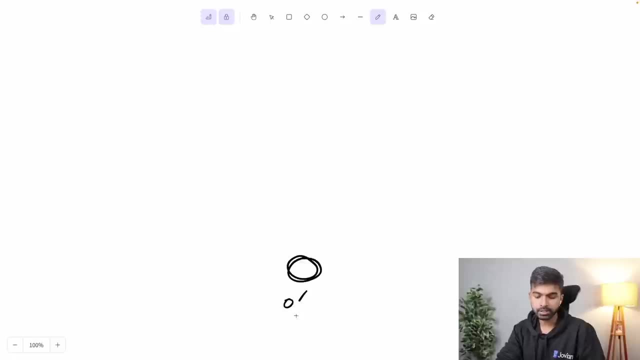 So here we have: Okay, These are the origin main branch, So this is the- I'm calling it the origin main. Okay, And based on the origin main branch in each of our code spaces. So let's say, this is the code space or Akash, and this and this is the code space or Sydney. 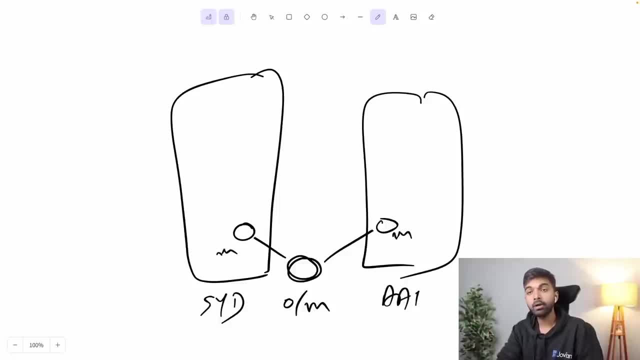 based on the origin main branch. Each of them has their own main branch. What Akash did was first make a change to the main branch directly and then push that back to origin, So that's how origin got updated. Okay, Then Akash has created a feature branch and then created a pull request from the feature. 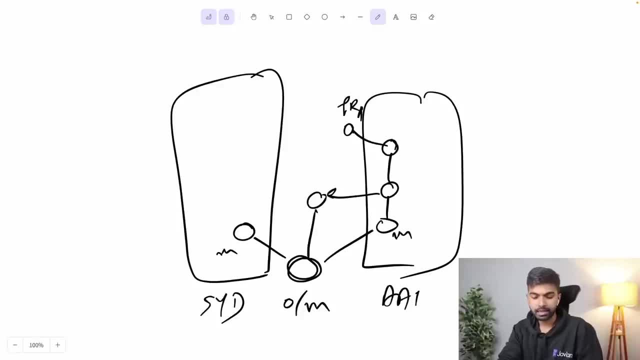 branch called PR one. Then Sydney, based on the old version of the new of the main branch, not using the new version of the main branch, made some changes and created a pull request called PR two. Then we merged the changes from PR one into the main branch. 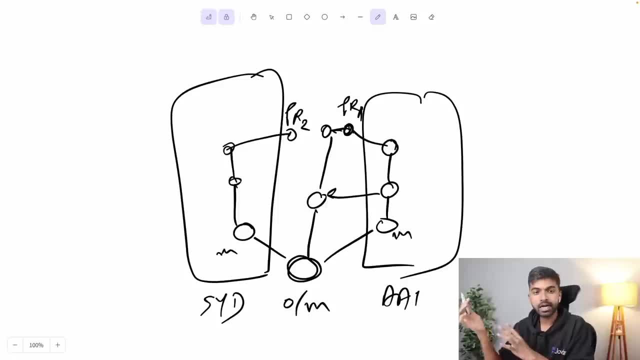 So this PR one is tracking. It's tracking a side branch and we merge those changes back into the main branch. So now the main branch is in conflict. These two cannot be merged. There's a conflict because both of them have edited the title. 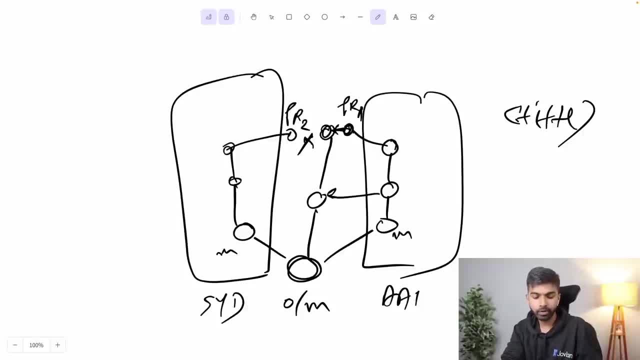 So then we tried to- here's what we try to do- into our main branch. We try to pull in these changes into our main branch. here We tried to pull in our changes and we tried to get a new version of the main branch. 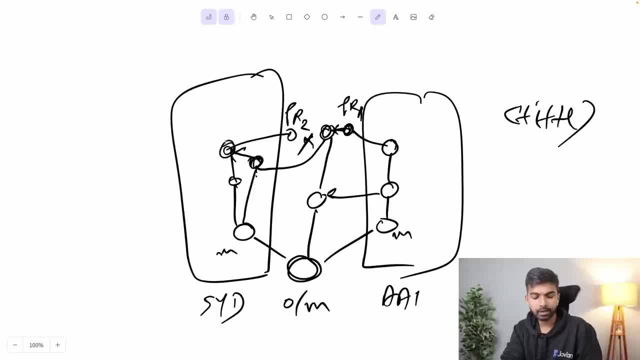 Okay, We tried to merge those new version of the main branch back into our feature branch- And that is when we resolve the merge conflict- And then we pushed our feature branch back And now the feature branch was compatible with the main branch And so these could be merged together. 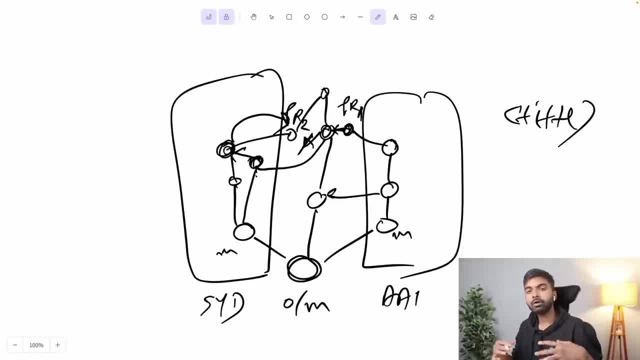 Okay, I know it's confusing. You have to work it out on paper by yourself. You have to try to create a couple of pull requests. You can also go through this explanation again, But only when you do it, you realize it. 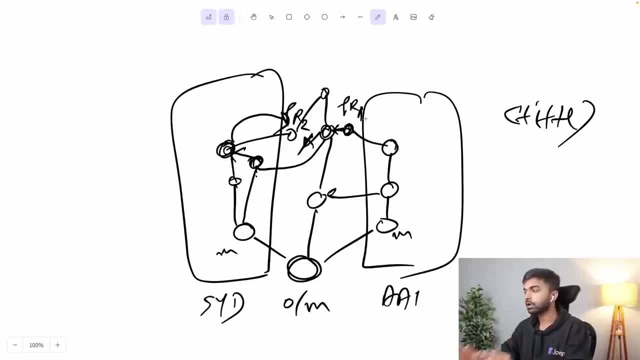 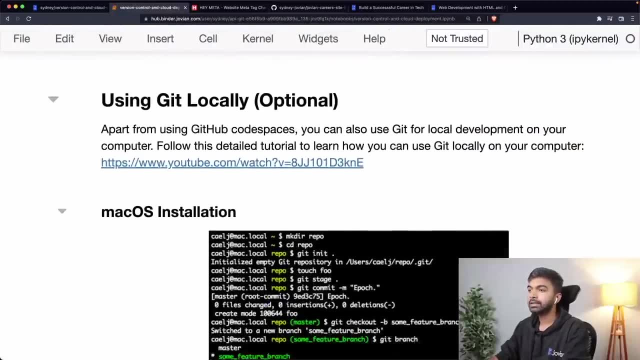 But, all said and done, What we've been able to achieve is we've been able to resolve a merge conflict. All right. So that is the final topic that we're looking at today: Resolving merge conflicts. There is another optional topic on using Git locally. 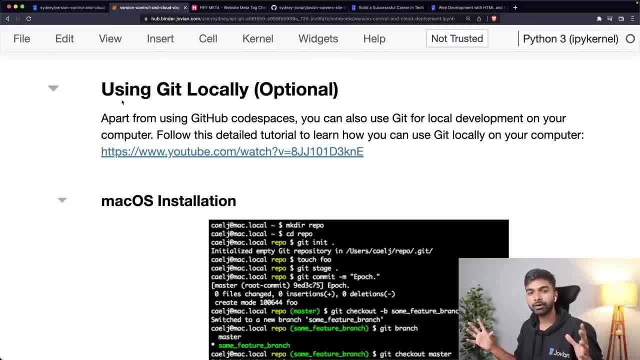 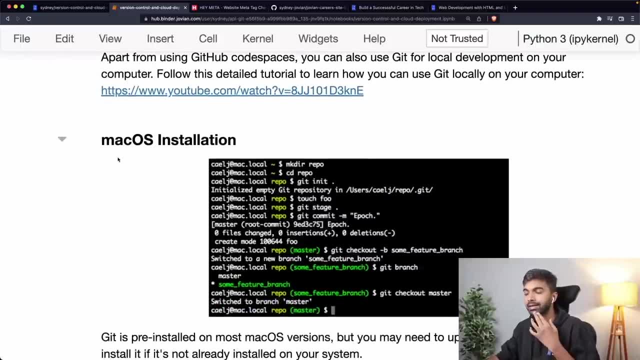 I will not get into it today because we've covered a lot of material already. We have looked at a bunch of different things, but there is a way for you to use Git locally. What you can do is you can download Git on macOS or on Windows or on Mac. 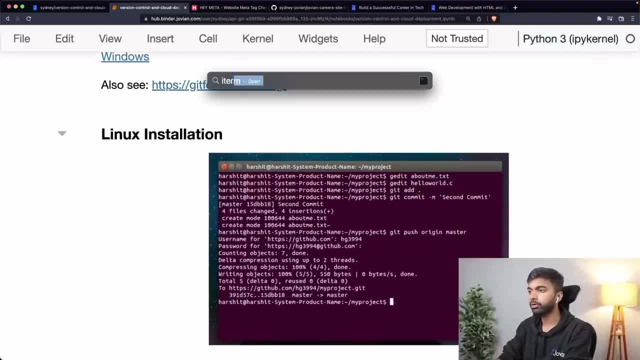 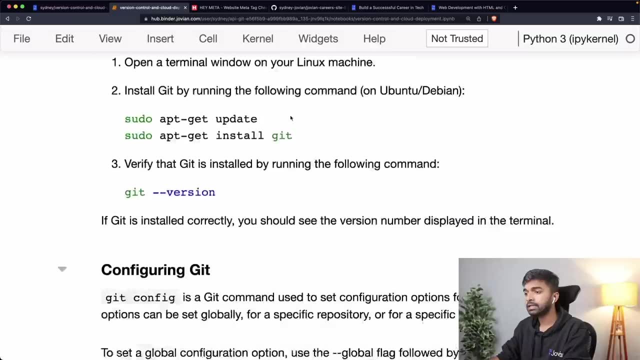 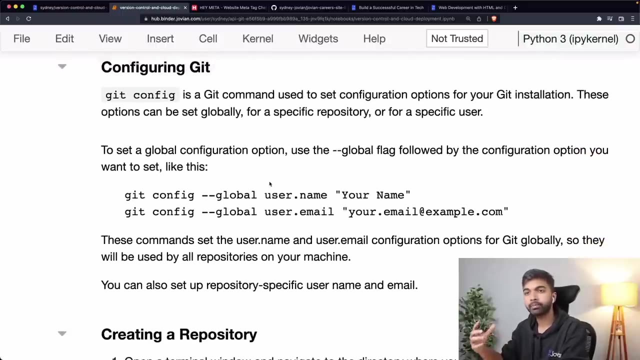 Okay, Linux. So you'll get this Git command line tool on your computer. It will look something like this: Git minus- minus version. It will show you Git. Okay, Then you can. actually you'll need to configure Git, So you need to configure a username and you'll need to configure an email before you can start creating repositories, making commits. 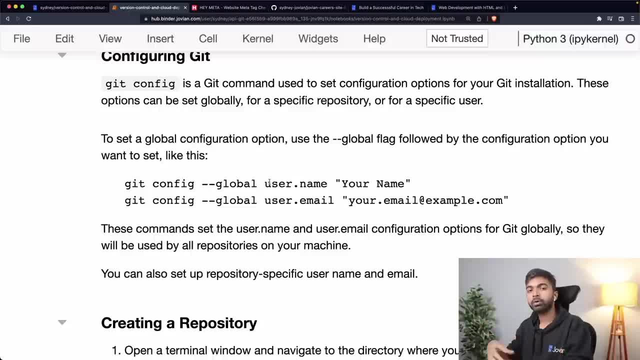 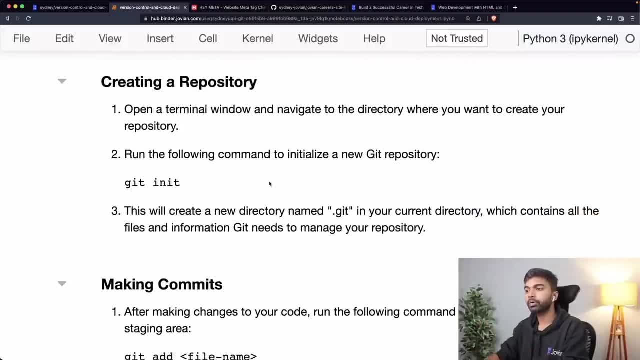 Now what you can do is you can either create a repository and push it to GitHub, or you can get an existing GitHub repository down onto your computer. If you want to first create a repository on your computer, That is done using the Git init command and that will create a new directory called git in your present working directory. 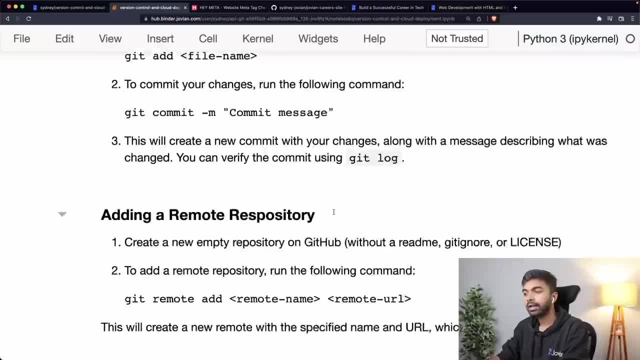 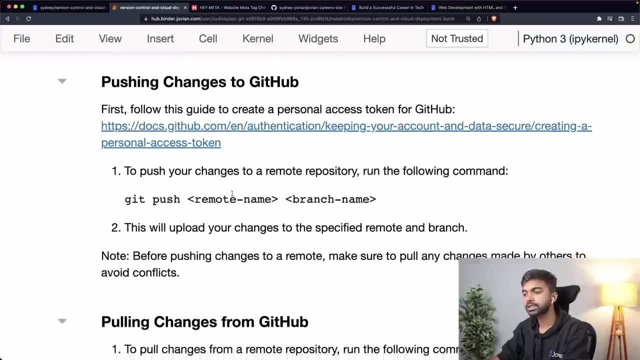 And then you can make commits locally on your computer and then you can add a remote repository on GitHub and you can then push your changes to the remote repository. So there are some instructions here and you can also, if other changes are made on the repository online, you can pull those changes back. 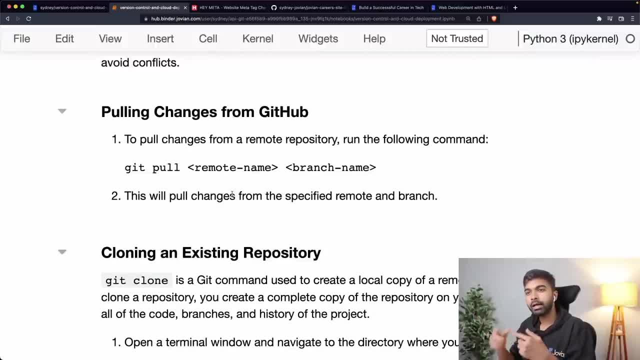 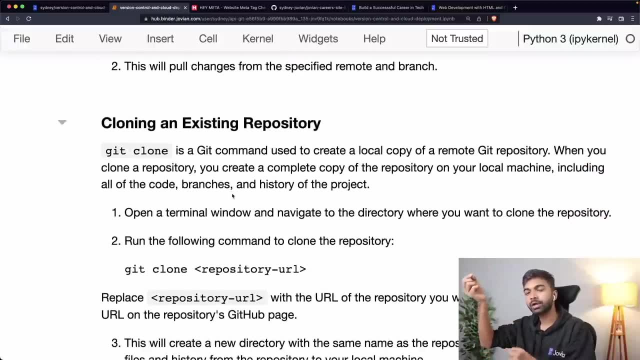 Okay. So that's one flow where you create a repository on your computer, add some commits to it and push it to GitHub. The other flow is that there is an existing repository on GitHub. in that case, to get the first version of that repository, you do something called a Git clone. 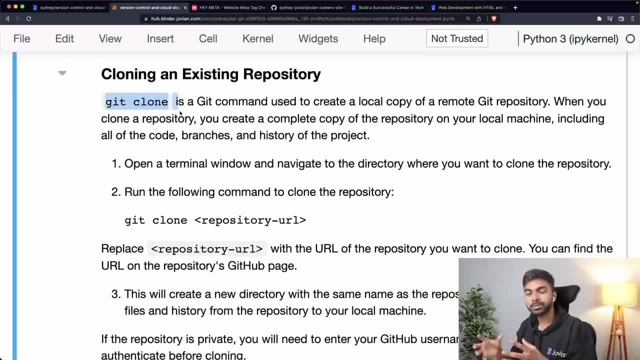 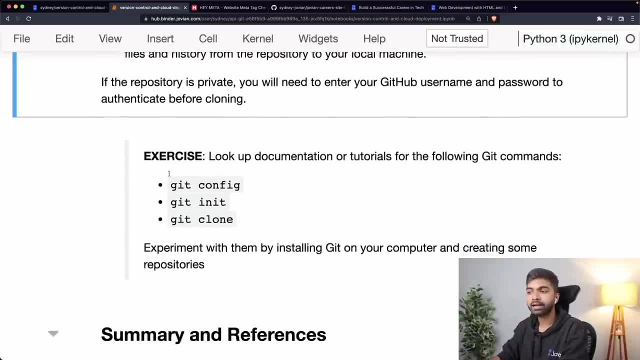 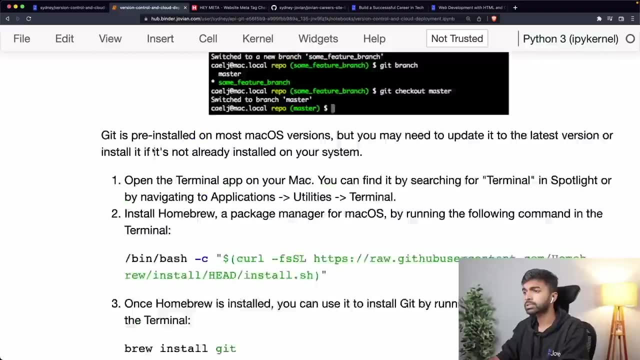 It's a more terminology. Uh, you clone that repository, which means you get your first version of that repository, Then you can make commits into that repository and then you can push that repository back onto the cloud. Okay, So I've linked to a tutorial here that you can go through in case you want to use um, in case you want to use GitHub on your computer. 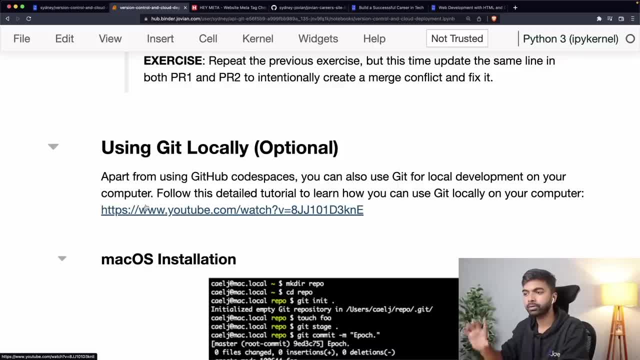 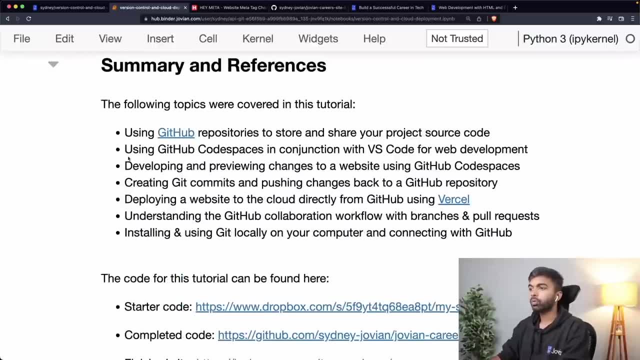 So follow this YouTube tutorial. It's about 40, 50 minutes long and it'll get you through all of these as well, But here is where we are going to wrap up today. So here's what we looked at. We looked at using GitHub repositories to share your project source code, and the simplest usage is very simple. 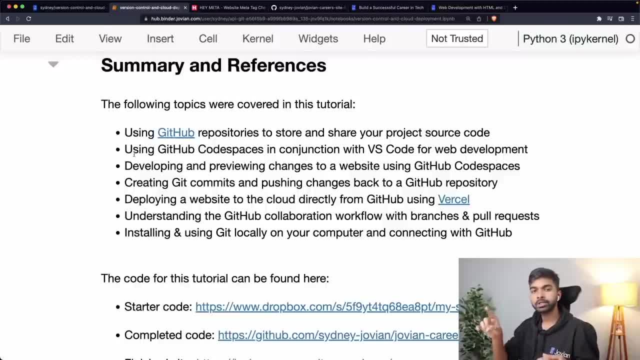 You go on githubcom, you click create repository, put in some information, add a readme file, add a gitignore file, add a license file and you create a repository. Very straightforward, right? So the simplest way to create a repository is just to go on githubcom and create a repository. 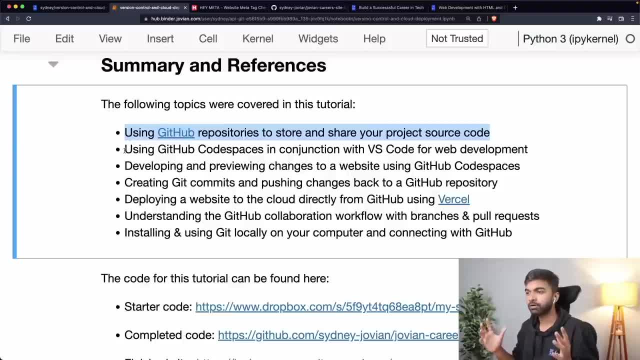 Then opening up a GitHub repository on code spaces is also very straightforward. You just go onto the repository, place a page, you click the code button and you say: edit in code spaces. So till now there's no Git commands, even that you need to run. 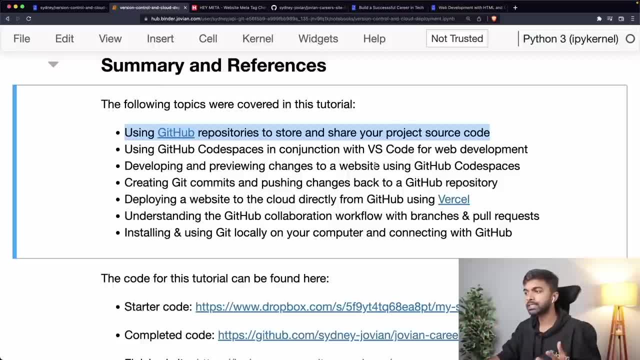 You just have to open up um a code space and you can use VS code for development. Then, while you're developing the website, uh, use Using code spaces, you just make changes. You can upload files or you can create new files and you can add code within those files and you can then preview them using the live server extension on Git. 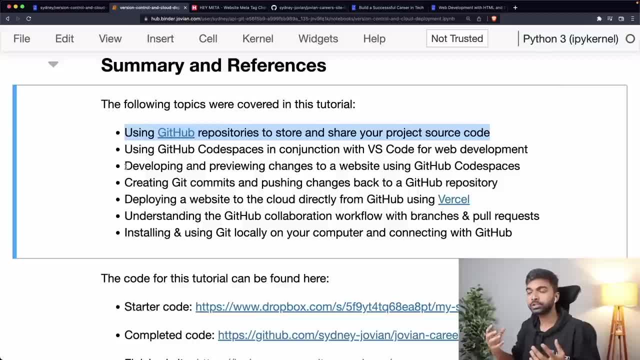 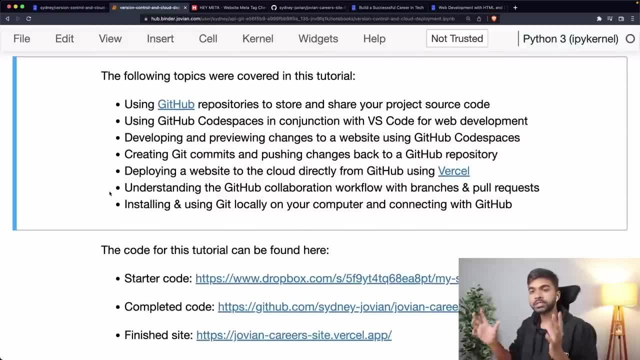 So the live server extension within VS code can let you preview changes while you are developing. That is again fairly straightforward. The next step now? all of this is still happening on the main branch. The single branch that you get is to create Git commits. 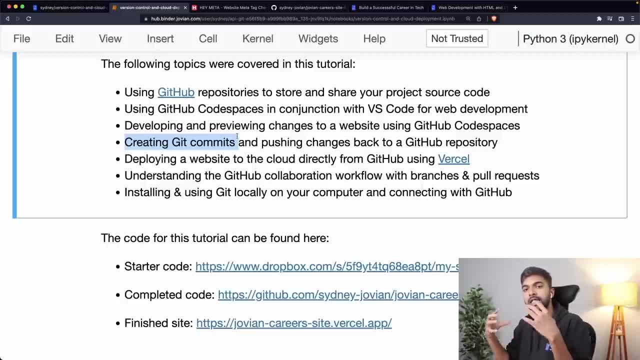 So what do you do is you take some changes You've made, You first stage them and then you stay. then you take those stage changes and then you commit them, So you record a version, a new version, locally and then you push those committed changes back to GitHub and that way the GitHub repository gets updated. 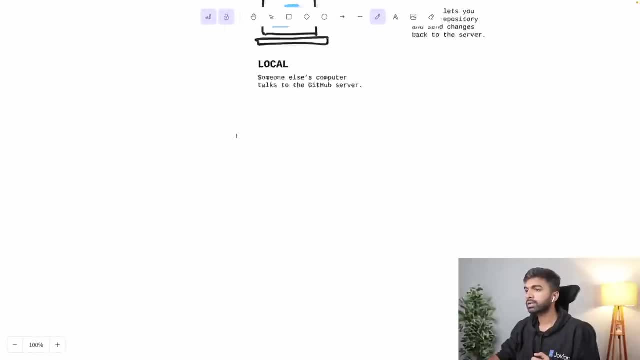 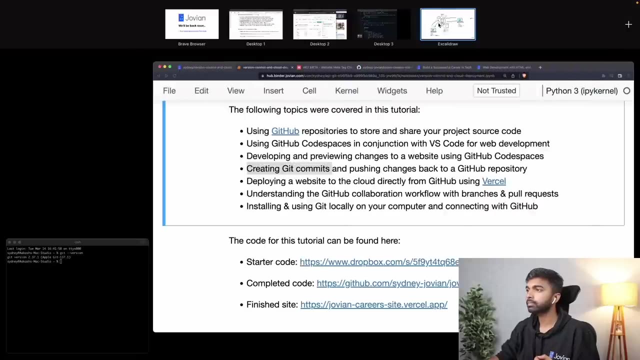 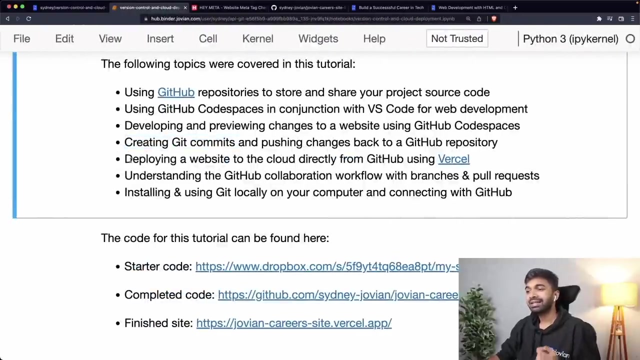 So always remember this, always remember this picture. What you do is you do some local development and then you push the changes back into the remote server. You push the changes back into The remote server, which is GitHub. Okay, Then we learned how to deploy a website to the cloud directory from directly from GitHub using Vercel. 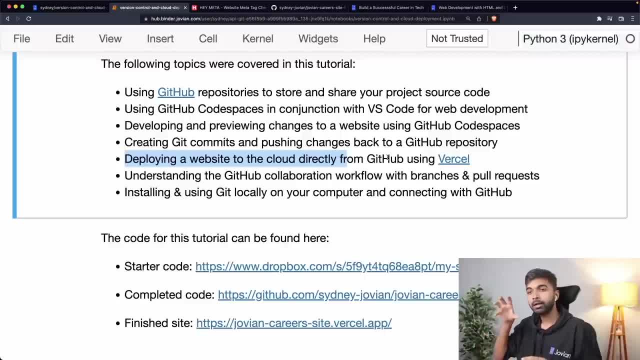 And again, it's really simple. You just go to Vercelcom, sign in, connect it to your GitHub repository and then just click deploy, And every time the main branch is updated, which means every time you push some changes into the main branch- then your repository is going to get updated and your website is also going to get automatically deployed. 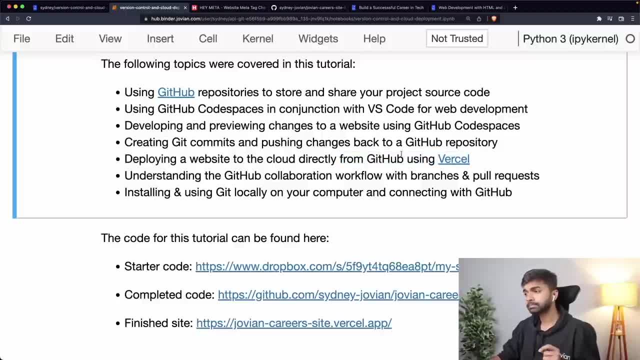 Very easy And you can also connect a custom domain if you want. So all of this is largely enough for working on personal projects. but we also have the GitHub collaboration workflow. So what happens in the GitHub collaboration workflow is that on your code space you take a branch out, you make some changes within the branch, you make some comments within the branch, you push that branch to GitHub. then you set up a pull request. 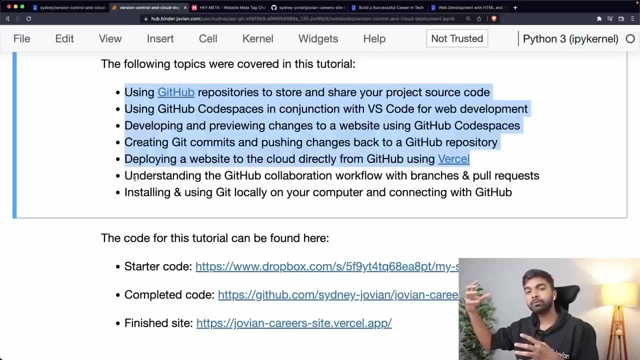 And once you set up that pull request, then somebody else can review that pull request And Vercel also creates a sample of preview deployment without affecting your main branch And once that pull request is approved you can merge that pull request back and the main branch gets updated. 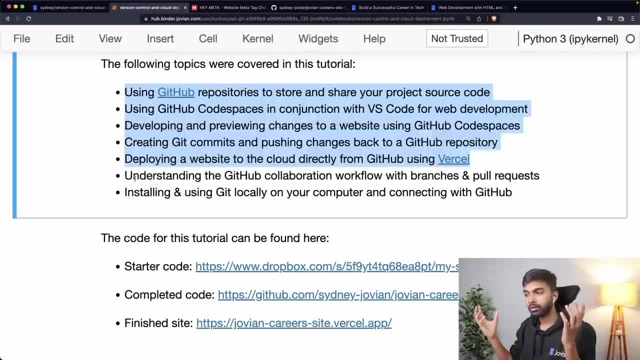 And so a new version of your project gets deployed automatically by Vercel. So that is a safe way for you to work on multiple features at a time without affecting the main branch, without affecting the main deployment, and whenever you're ready to bring things back, you can merge. you can approve that pull request. 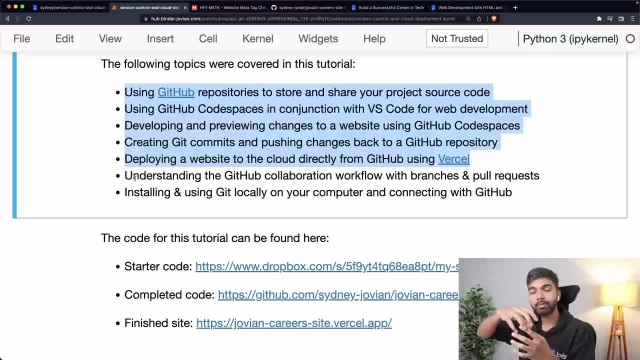 or somebody else from your team can approve the pull request and bring the changes back into the main branch. Okay, So that is the GitHub collaboration workflow, which is also fairly straightforward: Create a branch, make some commits, create a pull request, get it reviewed. 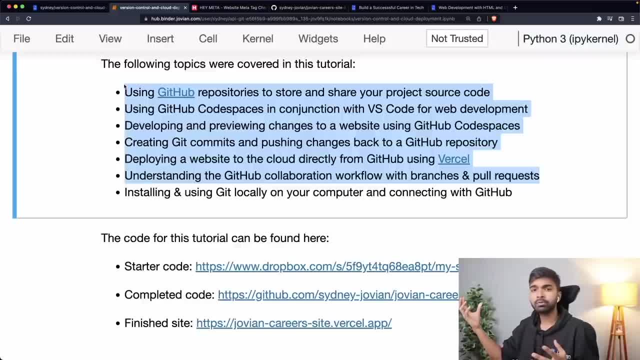 keep iterating on that branch And finally you merge those changes, after the pull request is approved, back into the main branch. Okay, Now where it starts to get complicated is when you have these merge conflicts, when you have to keep your branches up to date and you have to. 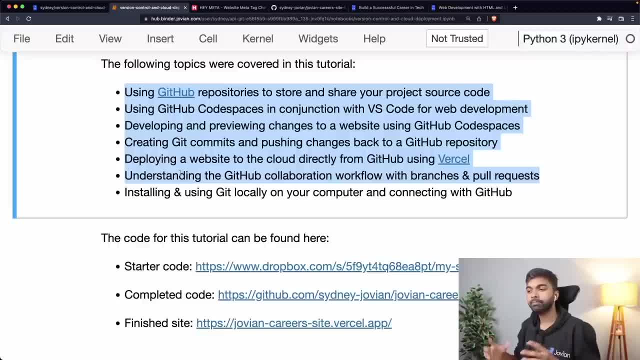 and there are conflicts where multiple people can have updated the same file. Now, although we've covered it today, don't worry if that does not make sense right now, because that's not something you're going to run into immediately And that is something that we are going to cover at a later. 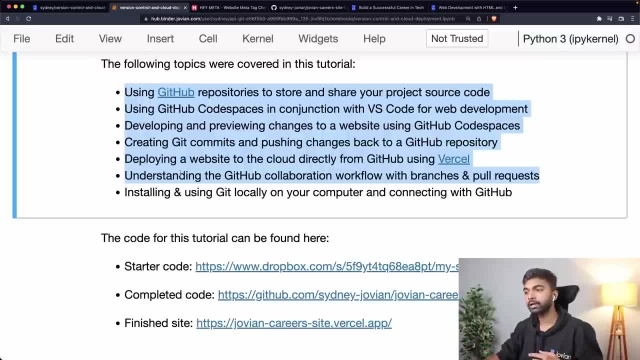 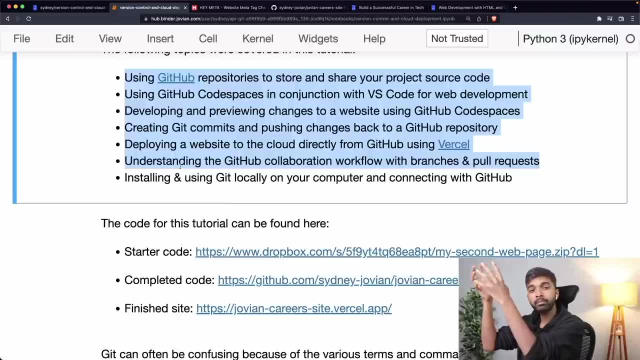 stage multiple times So you will become familiar with the flow over time. Okay, So that's it for this video. If you have any questions, feel free to ask them in the comments below. But how it works is you have to first get the latest changes from the main branch onto your 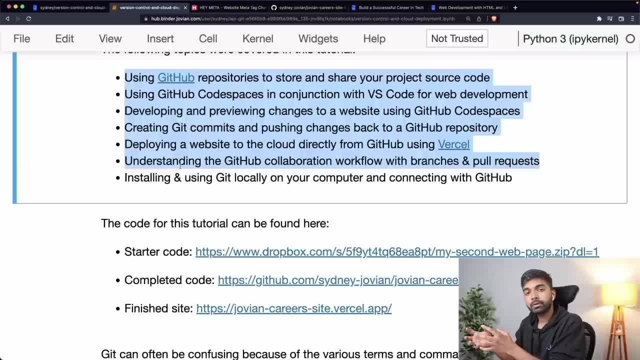 code space, then go into your feature branch and pull in those latest changes from main or merge in those latest changes from the main branch into your feature branch and then resolve any merge conflicts as they show up and push your feature branch back to update your pull request And that 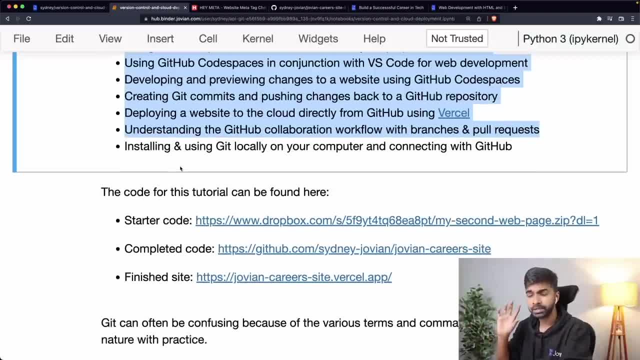 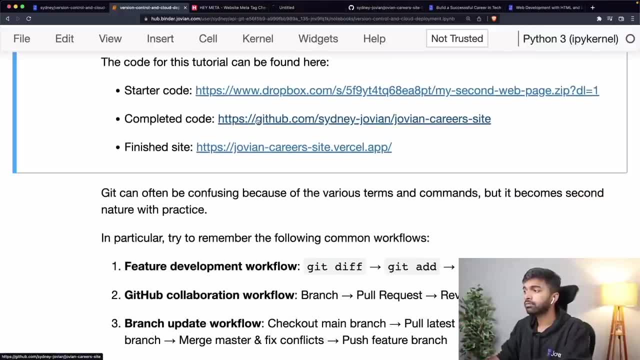 is how you keep your pull requests up to date. Okay, It's complex, no doubt, but only when you do it a few times you get used to it. So all the code for the tutorial is found here. you can find the. finally, from this point on, we'll just be using GitHub repositories, And you should also. 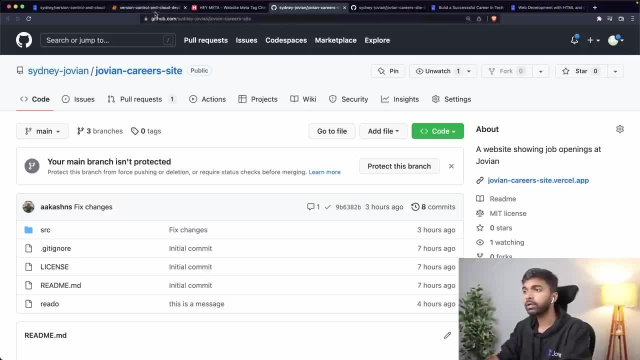 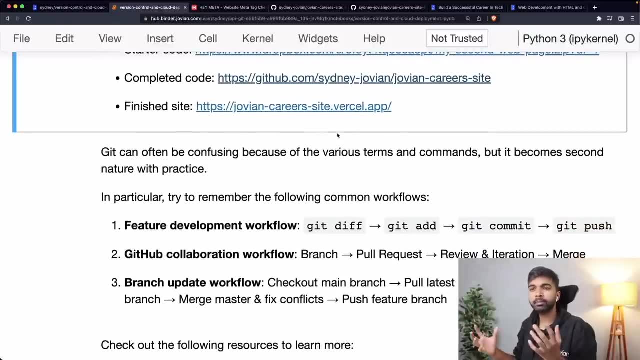 just be using GitHub repositories for all your work going forward, So you should do that, And you can check out the finished site here as well, which contains all the meta tags etc. in place as well. So we also looked at meta tags and how they can be used to set up a preview image. some 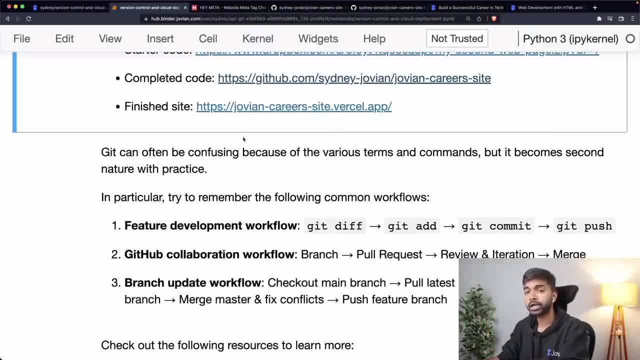 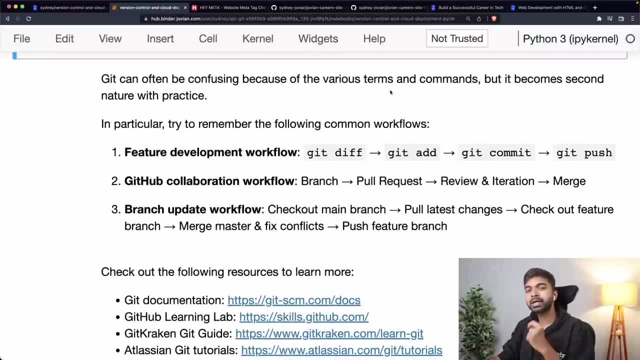 description and a preview title when a link is shared online. Now, get can be confusing because of all the various terms and commands, but it does become second nature with practice. I still look up commands on Git because, even after using it for 15 years, there are so many terms that I 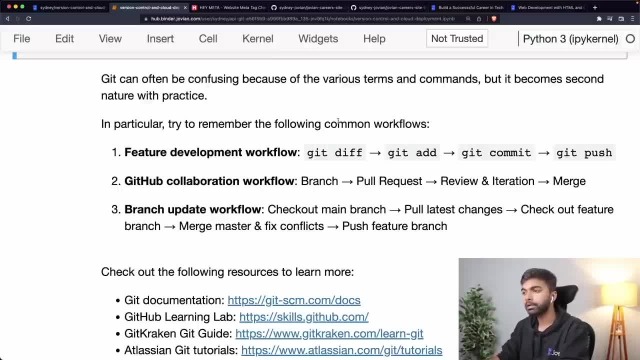 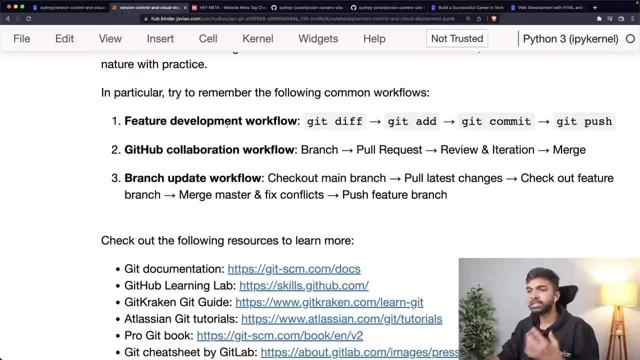 often find myself at a loss in terms of what I what I need to do. But, in particular, just try to remember these common workflows. when the simplest workflow is, you make some changes, you check those changes using git diff or using the Visual Studio Code API, you add those changes or stage those. 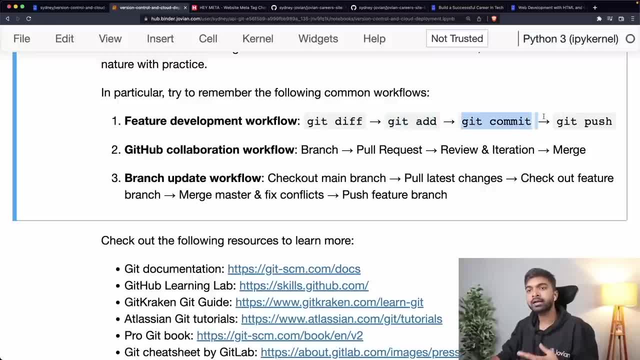 changes using git diff And then you can go ahead and set up a preview image And then you can do that dot, then you commit those changes using git commit minus m And then finally you push those changes to update your repository. Okay, this is what you should be doing right now. You don't need 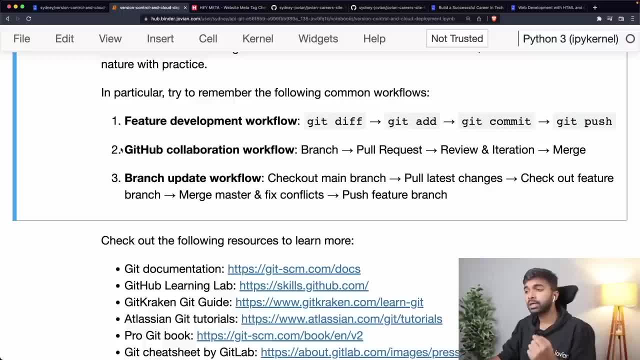 to do anything more than this. The next level two is understanding the GitHub collaboration workflow, where you create a branch and you make comments on the branch. you push the branch, you create a pull request for the branch to be merged into the main branch that is reviewed by other people. you 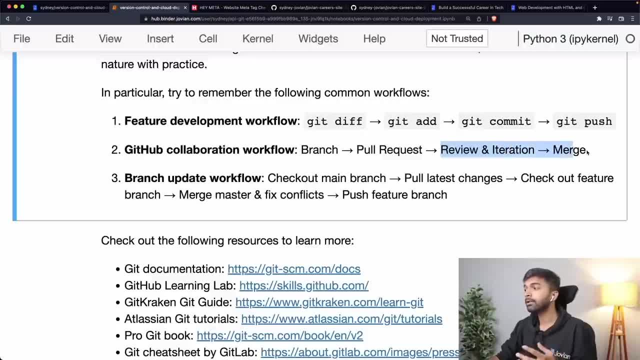 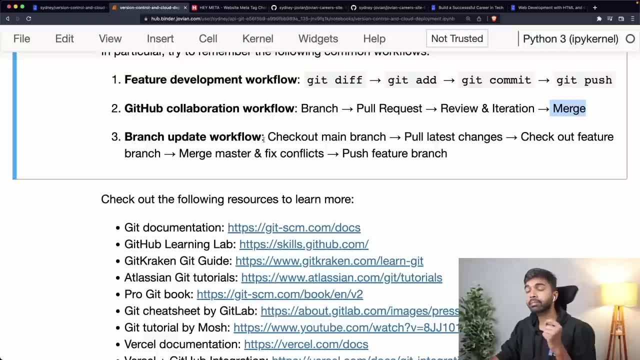 iterate, you make changes based on the comments and then you merge that back into the main branch. The third and the most complex workflow, which will take some time to get used to, is the branch update workflow, where you have to post whenever your branch has fallen out of date because the 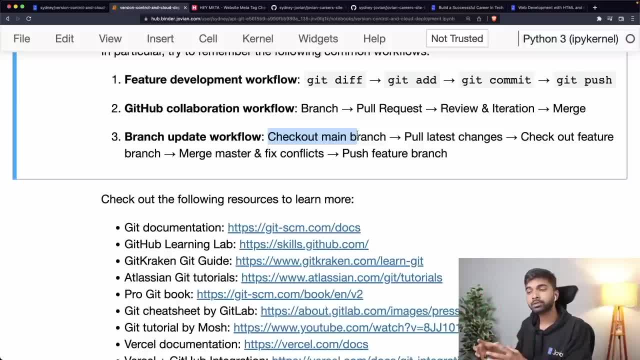 main branch has been updated a few times. First you go back to the main branch on your code space, get the latest change from GitHub, check out your feature branch, merge the main branch and fix any merge conflicts and then push the feature branch to update your pull request and you're good to go. 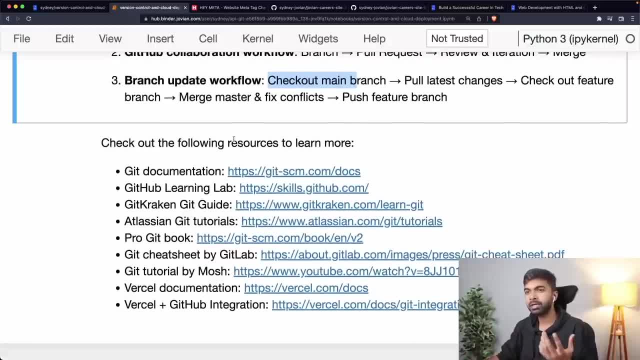 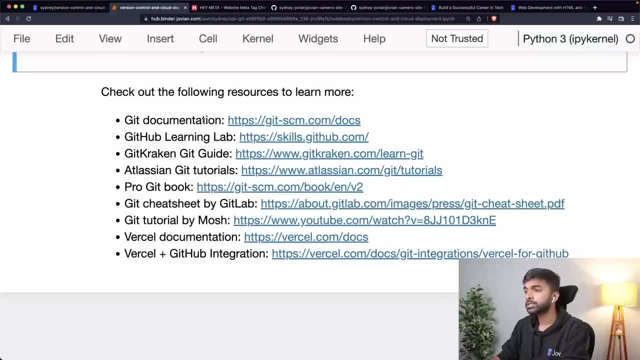 Okay, Try to practice it. try to set up a couple of accounts, or maybe even with the same account you can create two pull requests with some merge conflicts, and practice it, And here are some resources you can check out to learn more. So there is the Git documentation, of course, which 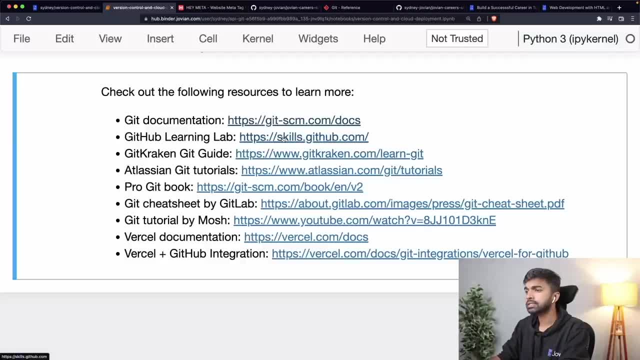 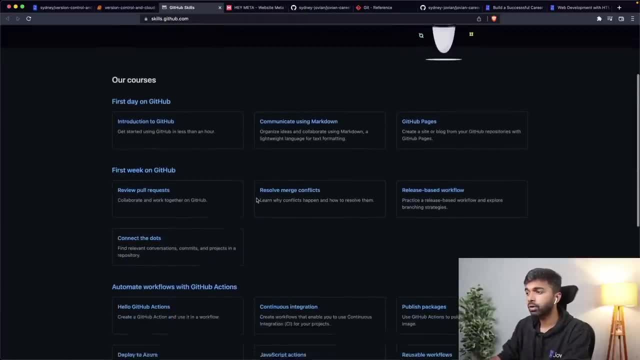 is the official documentation and reference that you can check out. There is the GitHub Learning Lab. So, specifically dealing with merge conflicts etc. you can check out GitHub Learning Lab. So all of this. you can see that there is this section on reviewing pull requests. there is this section on 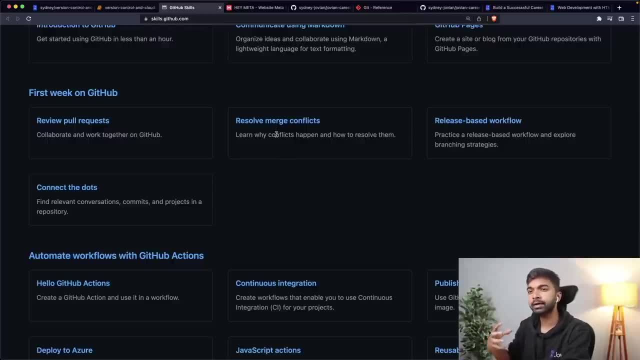 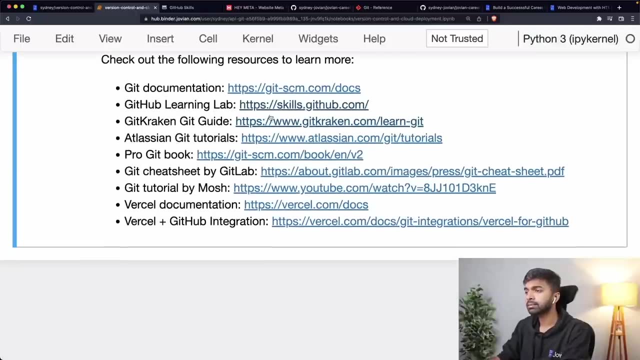 reviewing merge conflicts. So this will set things up for you in such a way that it will give you a starting point and then you will have to do some reviews, you will have to resolve some merge conflicts. There are some tutorials on Atlassian, some tutorials on Git Kraken. you can check out. 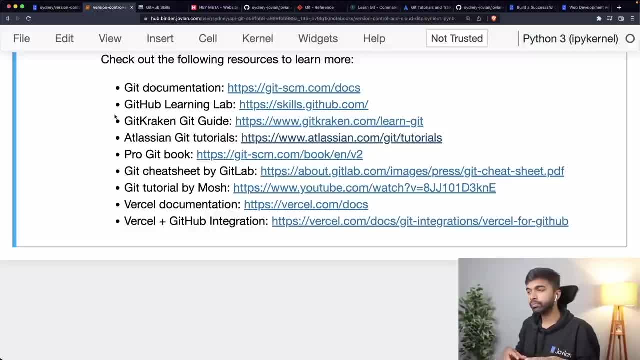 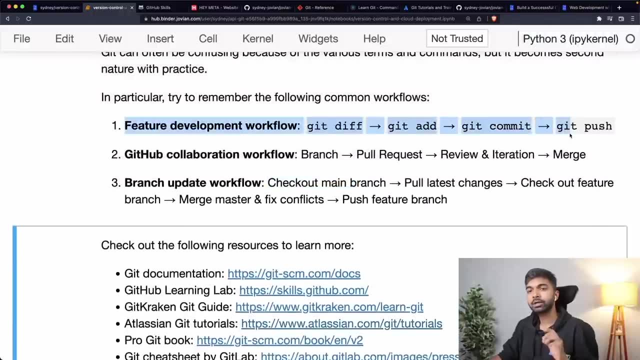 these as well. Again, Git is that kind of thing that you can keep exploring more and more. you don't have to become an expert on Git right away. If you can just do the first version, you are good to go. If you can do the second, that's great. 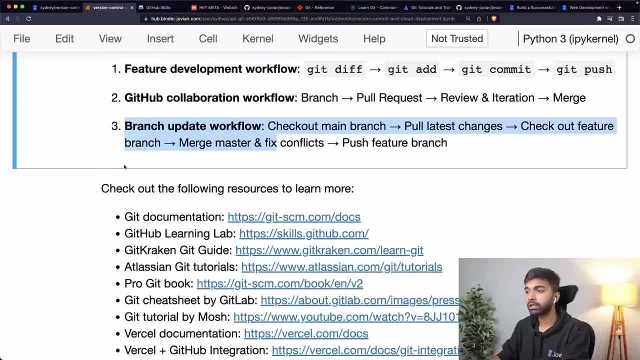 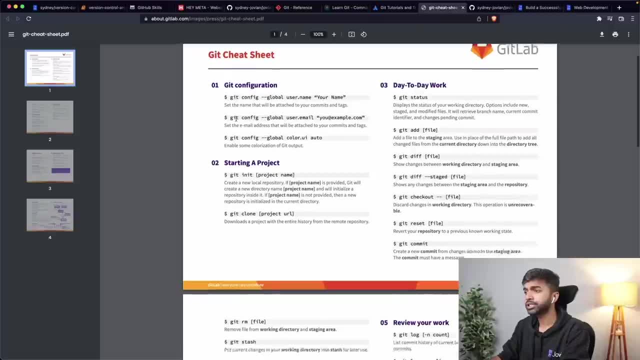 Over time, as you start working in a team, you will be able to start working on the third version or the third workflow as well. Okay, There's a Git cheat sheet by GitLab. You can go check out this cheat sheet. It contains some of these common workflows so that you don't have to think about. 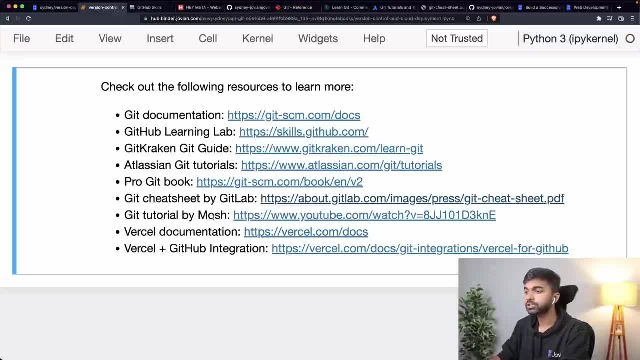 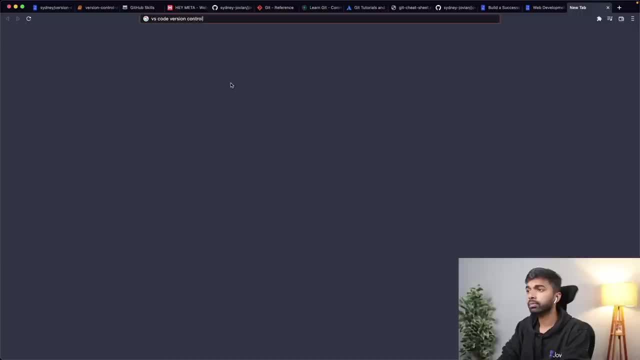 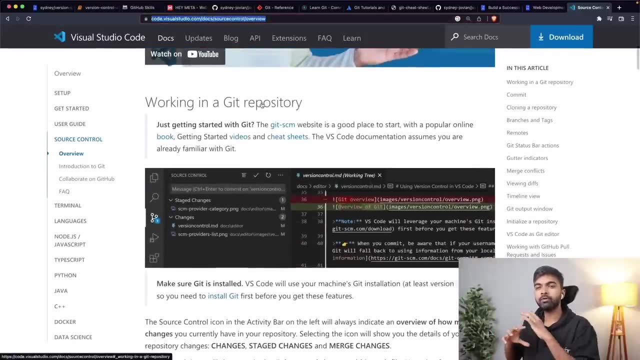 all the different Git commands together, And you should also check out the documentation for VS code. So if you just search VS code version control, you will find that there is this detailed set of videos and tutorials on how you can perform every Git related action directly within. 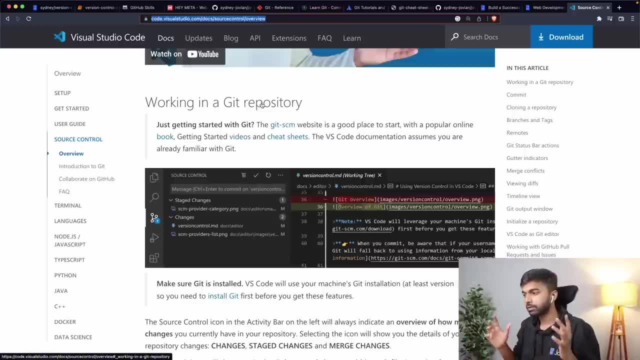 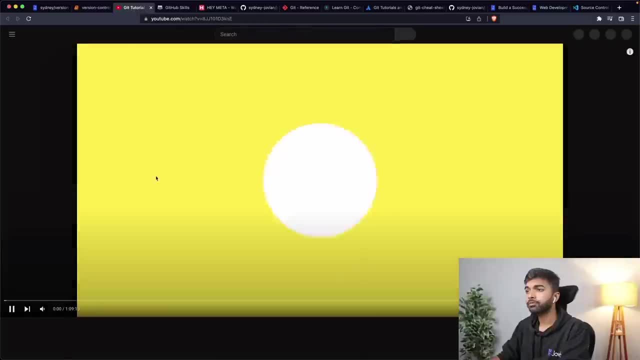 VS code without ever having to type a single command, So most of the time you'll just be using this at work, So check this out as well as well. There is this nice YouTube tutorial that you can check out for a for local Git development. we did not cover local Git development because we are 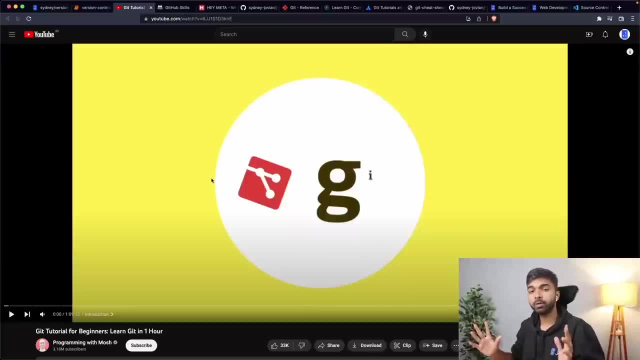 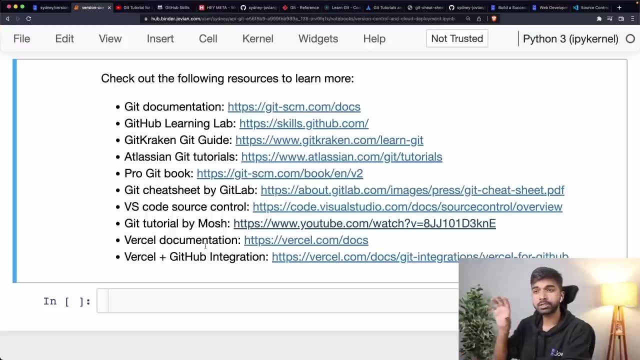 going to abuse. we are going to be using code spaces for the rest of this course and for the rest of this program as well. But if you want to do some local development on Git, we have some instructions on installing Git on your computer And then you can check out this. 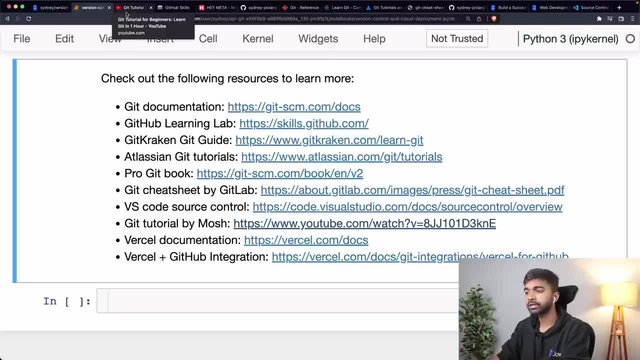 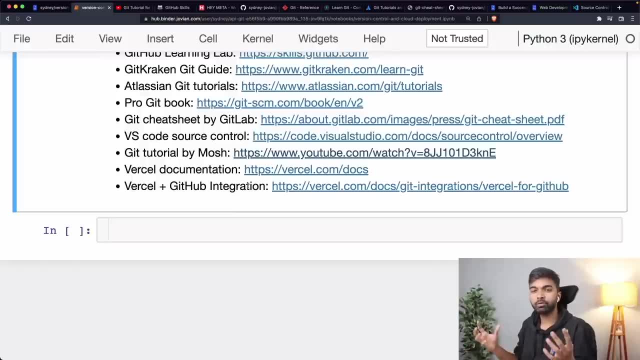 tutorial for things like Git config, Git init, Git clone, etc. Of course, you should check out the documentation for Vercel if you have more questions about how Vercel works. But the flow we've shown here, which is connected to your GitHub account: pull in the GitHub repository code. select the. 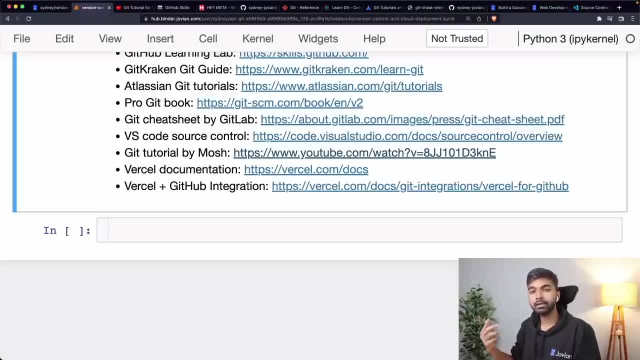 root folder and just hit deploy And then automatically, anytime the main branch is updated, it's going to create a new deployment, And anytime you create a pull request, it's going to create preview deployments that can be used for testing without affecting the main deployment, And then anytime the pull request gets merged. 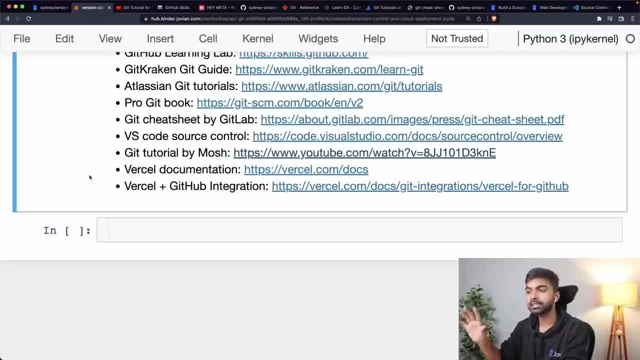 the main deployment gets updated automatically, So it makes things really seamless, And it is used in production. that is what we're going to be using extensively in this program, And you can learn more about the Vercel and GitHub integration here as well. Responsive design is a crucial 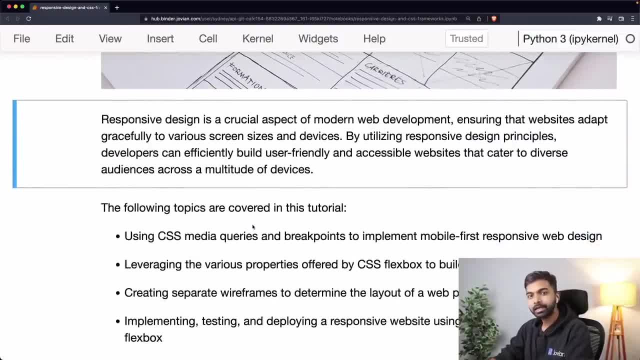 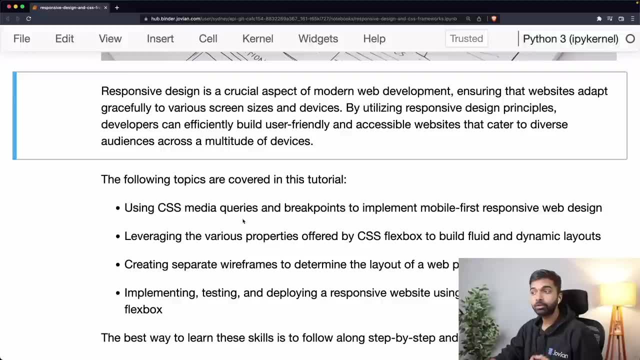 aspect of modern web development and ensures that websites adapt gracefully to various screen sizes and devices. And by utilizing responsive design principles, you can effectively build user interfaces and accessible websites that can cater to a diverse set of audiences from any set of devices, And in fact this is important. 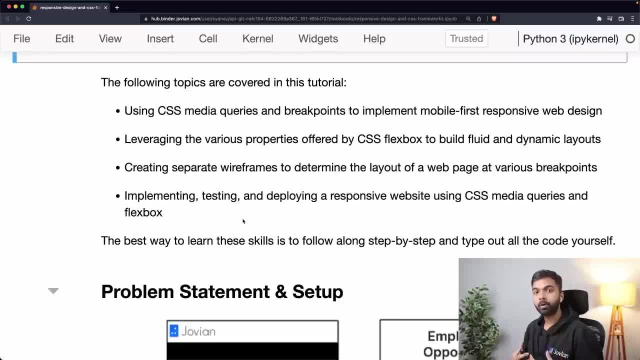 because over 70% of web traffic today comes from mobile and maybe another 10% from smaller tablets, And there's only about 10% of traffic that comes from the large desktop screens that we typically develop our websites on. So there is a bit of a disconnect in terms of what developers look at when. 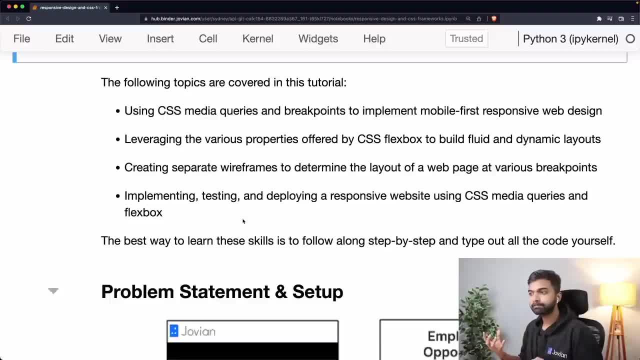 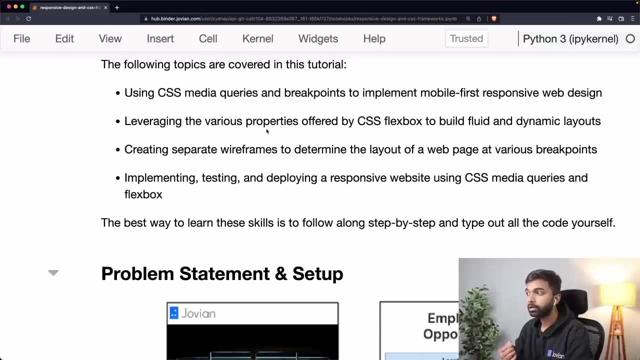 developing websites and what people look at when they're actually browsing these sites. So we'll talk about using CSS media queries and breakpoints to implement a mobile-first and responsive web design. We will also talk about leveraging the various properties offered by the CSS Flexbox layout model to build fluid and dynamic layouts. We will then learn how to create separate 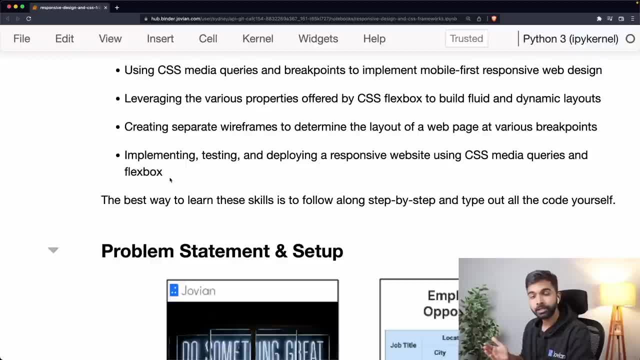 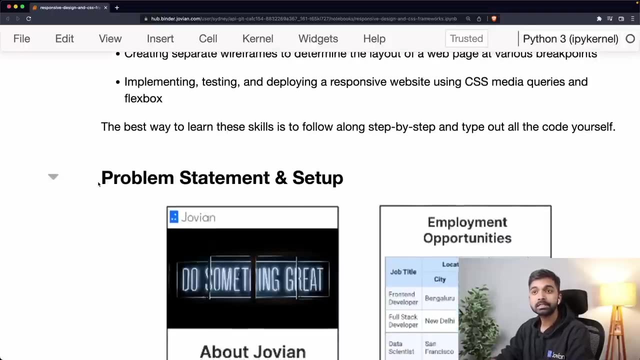 wireframes to determine the layout of a web page at various breakpoints, And this is how designers will often share designs with you. And finally, we will talk about implementing, testing and deploying a responsive website using CSS media queries and Flexbox. And, of course, the best way to learn these skills is to follow along step. 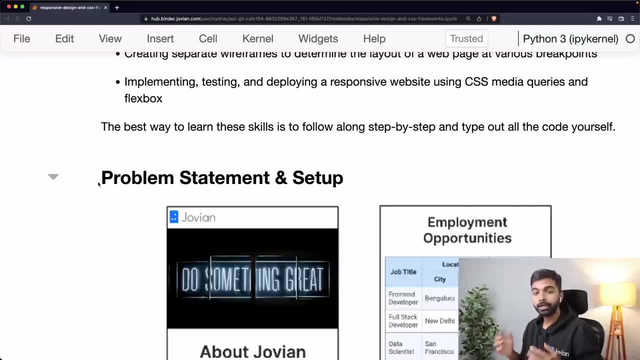 by step and type out all the code yourself. if you are not been doing that, If you have not been typing out all the code yourself, you're making a big, big mistake. It is going to severely slow down how much you're going to learn. 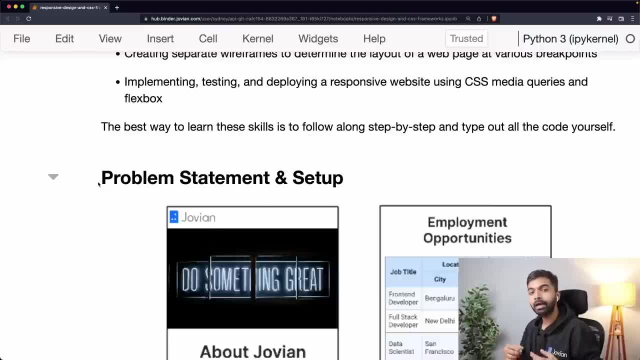 So type out all the code yourself, question everything that you do And if you get stuck at some point, please ask us. we have also just added a lot more one-on-one support call slots, And we're also decreasing the amount of time that we take to respond to your queries. 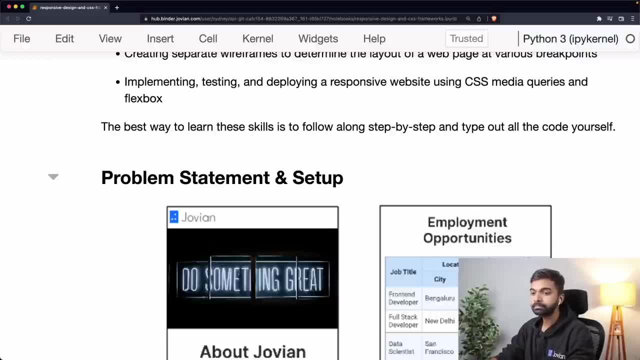 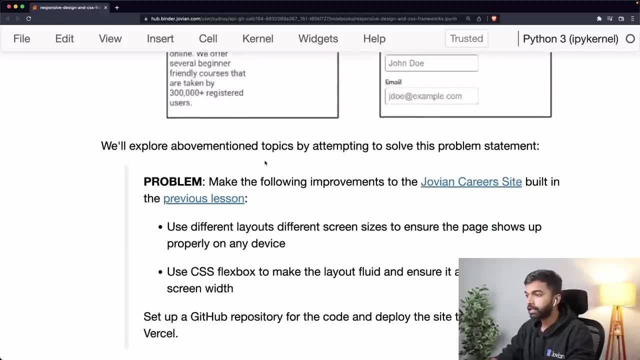 So please feel free to get all the help that you need. All right, So here's a problem statement that we look at today. Now, in the previous lesson we built a Jovian careers website, So this is what the website looks like. 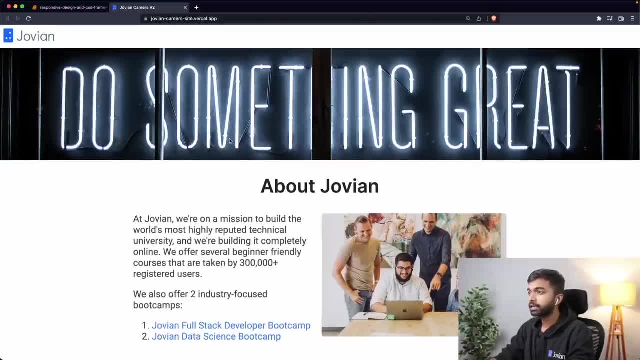 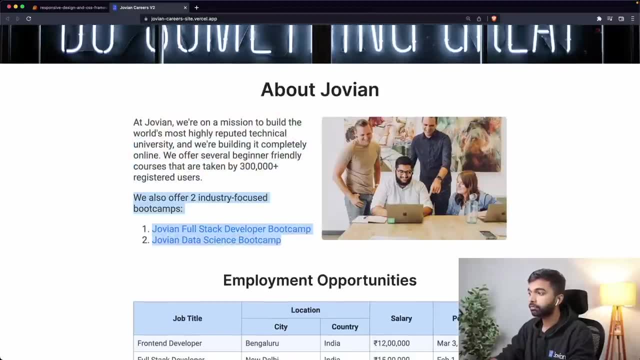 We have a navbar here With the Jovian logo. we have this banner image that says: do something great. We have an about Jovian section that talks about our mission and talks about two programs we offer, along with a picture. We have an employment opportunities table. 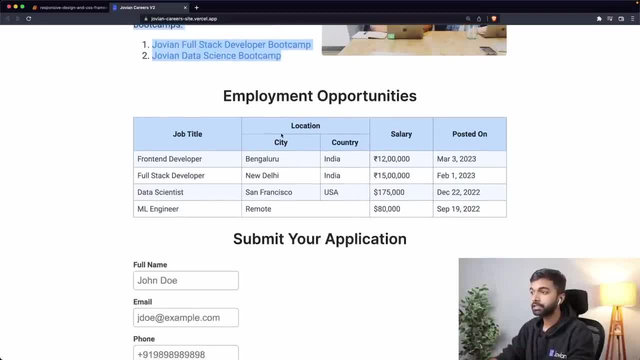 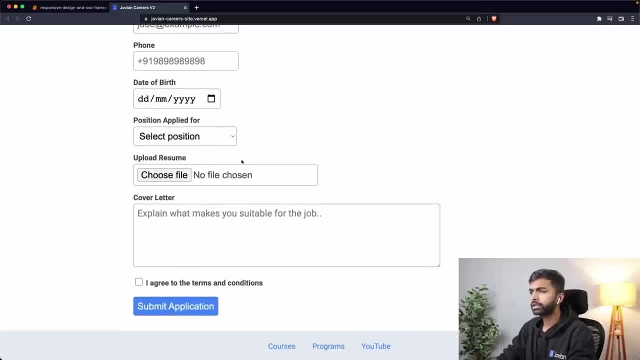 We found that a table was a nice way to showcase some employment opportunities, So that's great. And then we have this: submit your application form, where people can fill out their name, email, phone number, date of birth, select a position. upload a resume. add a cover letter. agree to terms and conditions. 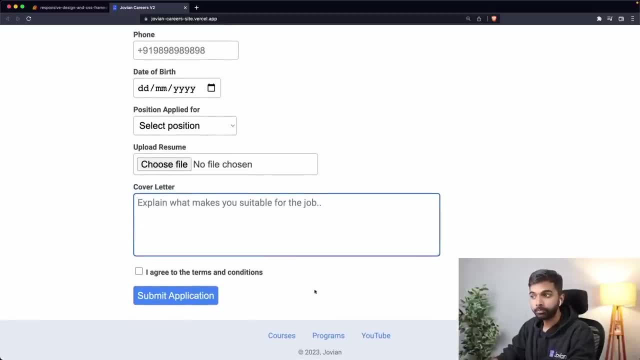 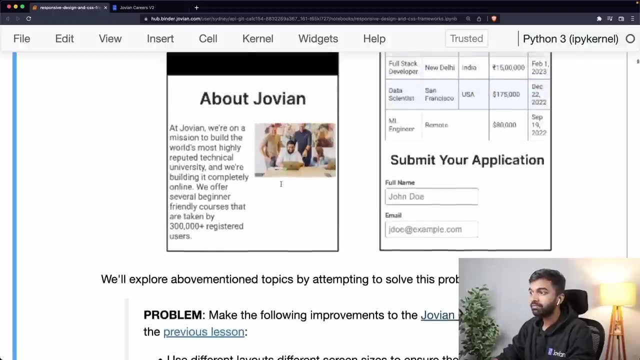 submit the application And finally, at the bottom, we have a footer. So this is the website that we have been developing step by step over the past few lessons. However, this same website, if you've tried to open it on mobile, you will. 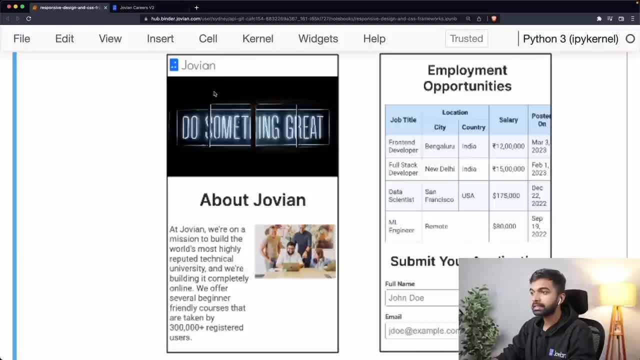 see that it doesn't really show up properly. What happens on mobile is this image takes up a lot of space. There's a lot of blank space above and below it. above and below this do something. great part. So we might want to reduce the height of the image on mobile. 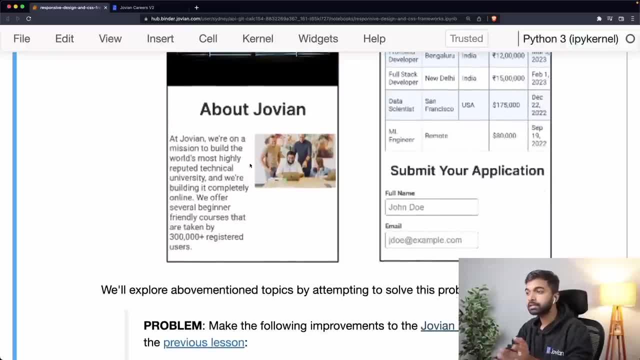 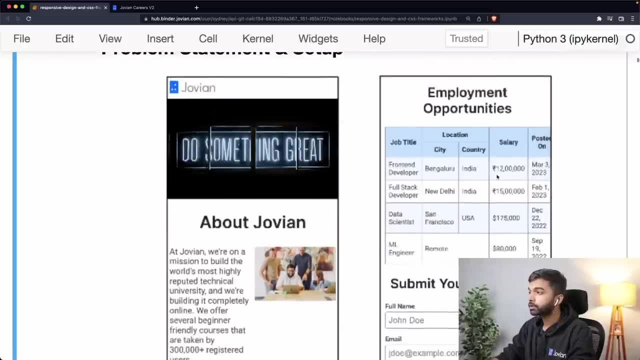 You may also notice that on mobile it doesn't really make sense to show these side by side, the text in the image. Maybe it'll be better to show the image below instead of on the side. Then you will also notice that the table does not show up completely on mobile. 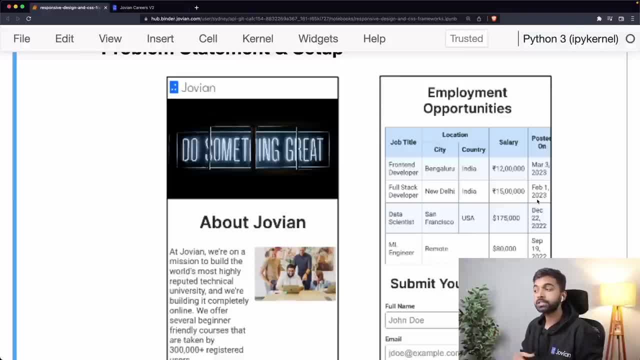 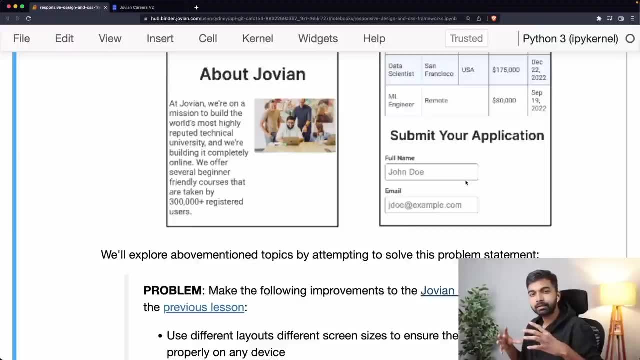 The table actually goes out of view and that requires horizontal scrolling, which is not a great experience on mobile. And finally, the application form as well. it feels a little cramped on mobile and it would be nicer if there was more space on mobile for each of the input fields. 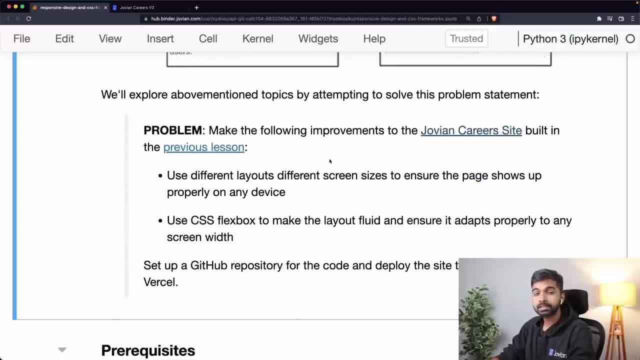 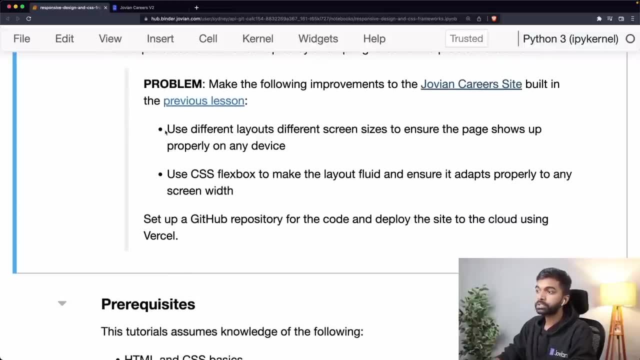 So We will try and improve This website to make it more mobile friendly, or what's called responsive. And here's what we're going to do: We are going to use different layouts for different screen sizes to ensure that the page shows up properly on any device. 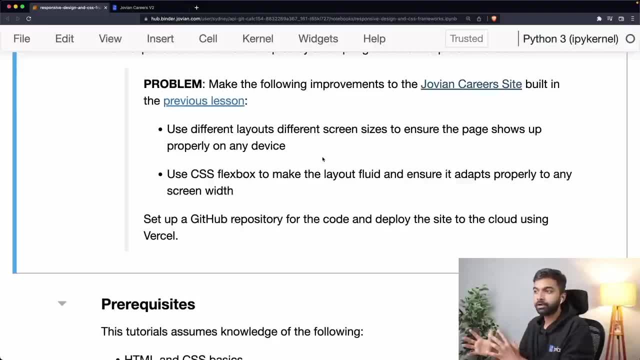 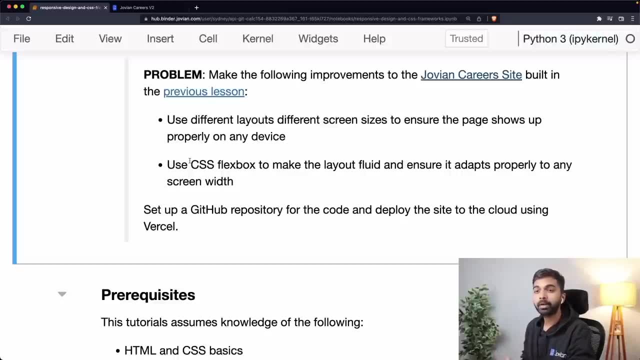 So it's going to look different on mobile, It's going to look different on tablets and different on desktops. We're going to use CSS flex box to make the layout more fluid and ensure that it adapts properly to any screen width, And we will also set up a GitHub repository- a new one, so that the old one is not. 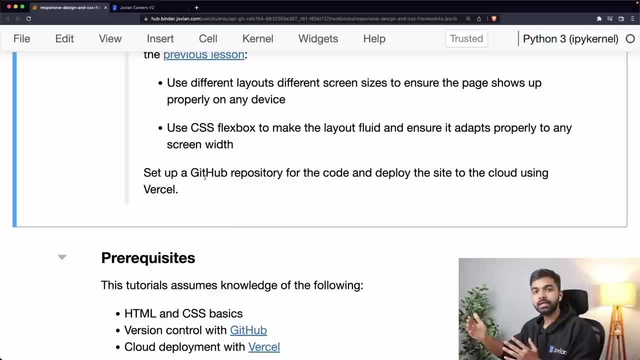 affected Now. normally, you will continue working on the same repository. However, just so that you have access to the old code as well, we will set up a copy of the previous GitHub repository and we will also deploy this new GitHub repository to the cloud using Vercel. 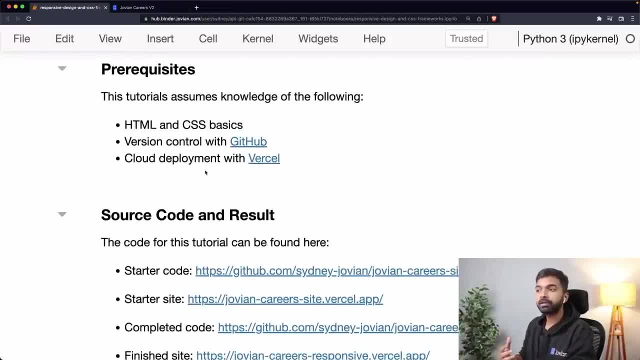 Okay, And of course, we are assuming here that you are familiar with the previous lessons, which is HTML and CSS basics, advanced HTML and CSS and version control with GitHub and cloud deployment with Vercel. The code for this tutorial, It can be found here. 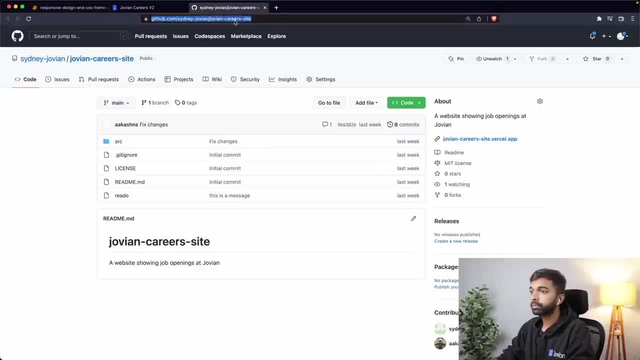 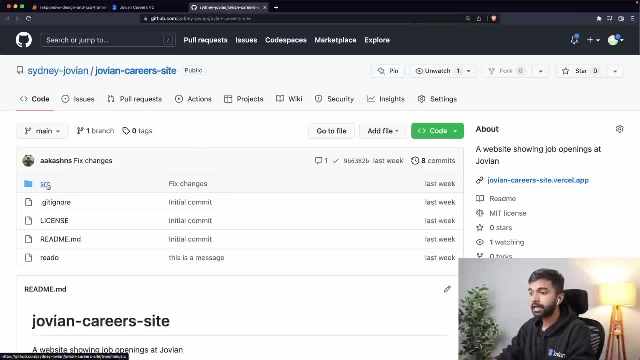 So this is the starter code. So I'm just going to open this up here. This is the. this is a GitHub repository which contains the starter code. You can see here that there is an SRC folder here and inside the SRC folder. 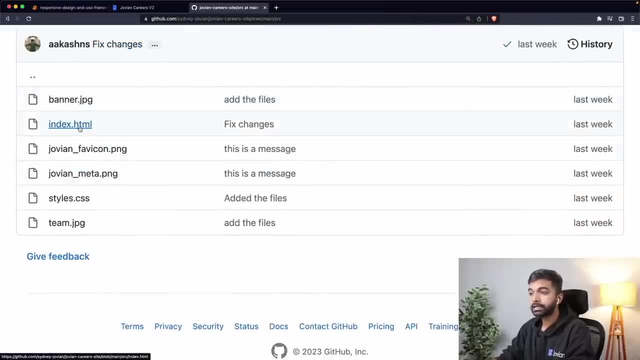 there is. there is an indexhtml file and there is a stylescss file. These contain the HTML and the CSS for this Jovian career site. Okay, You can also check out the The site, which is what we looked at just now. 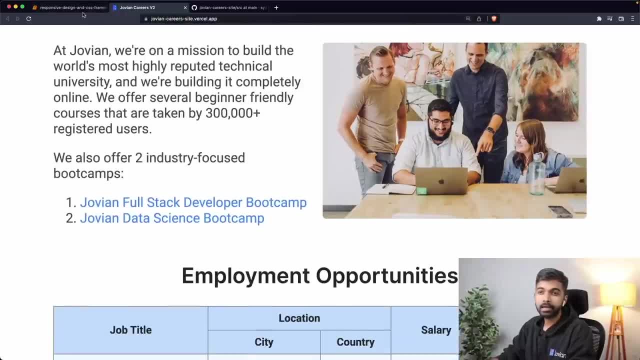 So this is the starter site that we are going to work on today, And I encourage you to take this URL and open it up on your mobile phone to ensure, to confirm that it actually does not look very good, so that you can compare it with the changes that we're making today and you can find the 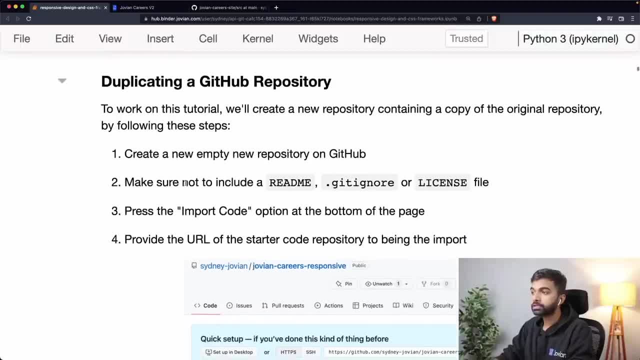 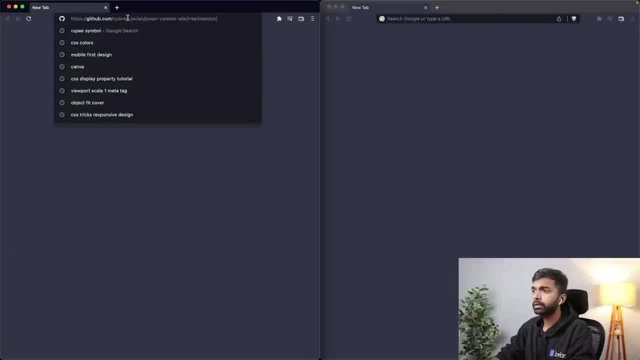 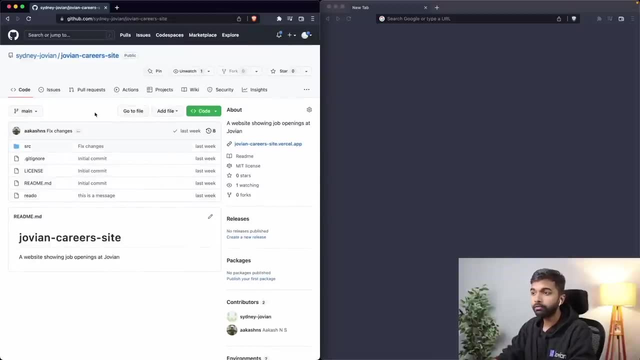 completed code in the finished site. here Now to work on this tutorial. we will create a new repository containing a copy of our original repository. Let us open it up here. Yeah, New window. So this is the repository that we want to create a copy of. 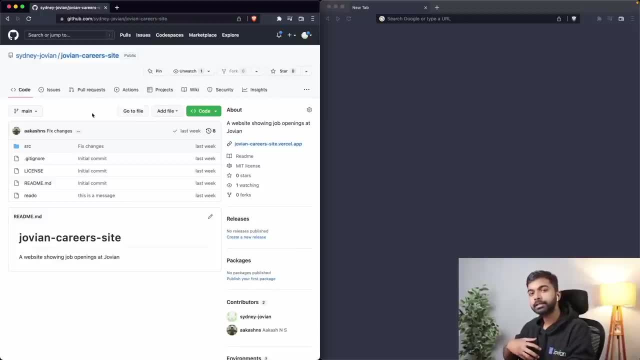 Okay Now, normally, if you want to create a copy of a repository that is owned by somebody else, you can just click this button called fork, and what fork will do is take the GitHub repository that is part of somebody else's profile and copy that. 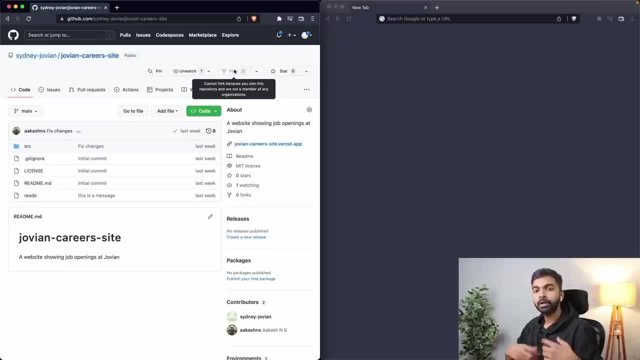 completely to your own profile as a separate copy, so that you can do your own development there. Um, but sometimes you have to fork your own Repository, and GitHub does not allow forking your own repository, So I'm going to show you a quick way in which you can create a complete 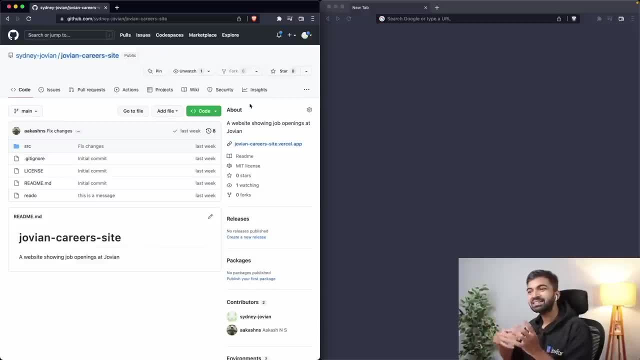 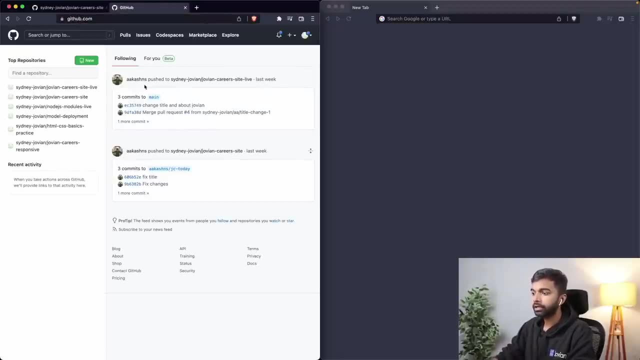 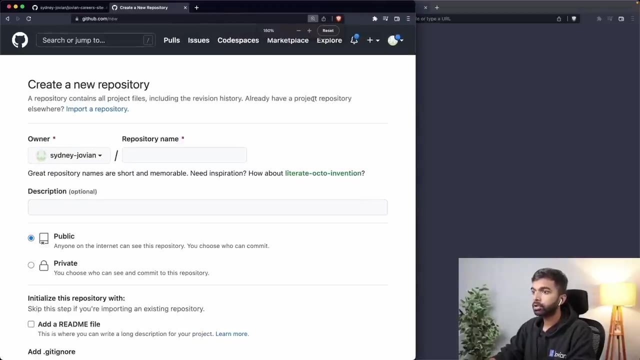 working copy of your GitHub repository as another new repository. So here is how we do that: Go to githubcom and on githubcom click the new button. here I'm clicking the new button And when you click the new button you will get the option to create a new. 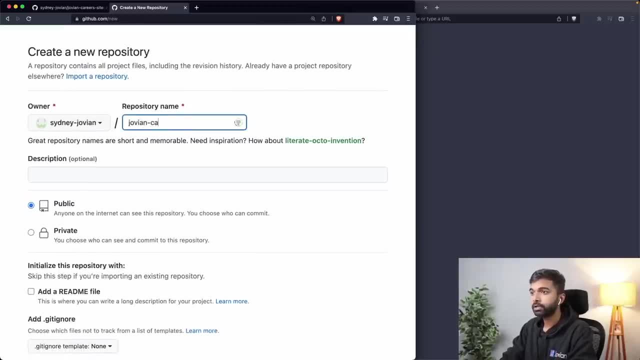 repository. So let me call this repository Jovian Career's responsive live, because I'm going to create a responsive or a mobile friendly version of this site and I'm doing this live, So I'm just going to calling it Jovian careers: the response of life a. 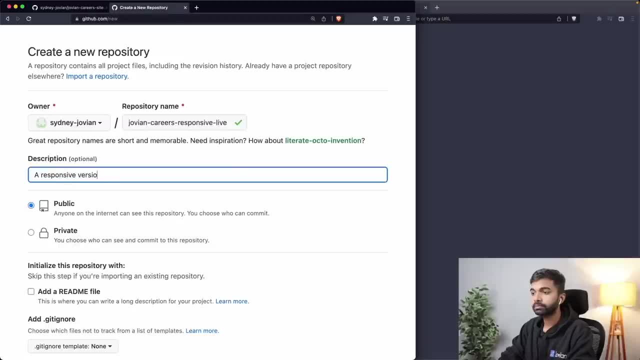 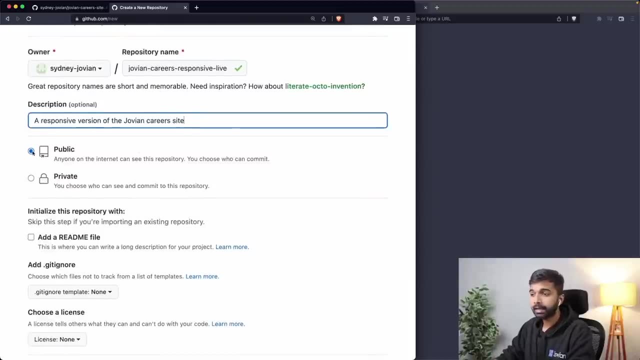 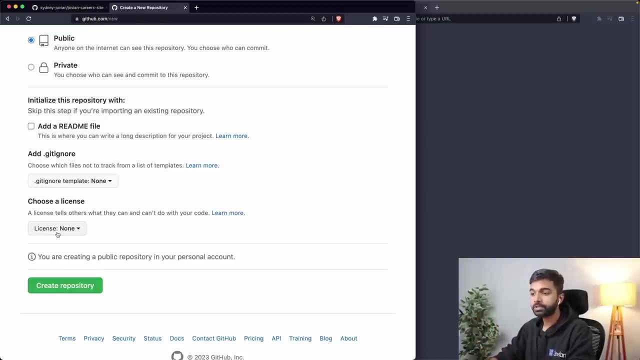 responsive version of the Jovian career site. Okay, I am going to leave this public and I'm not going to add a readme, gitignore or license. So this time I'm creating a completely empty GitHub Repository. So once I click create repository, now a completely empty repository gets created. 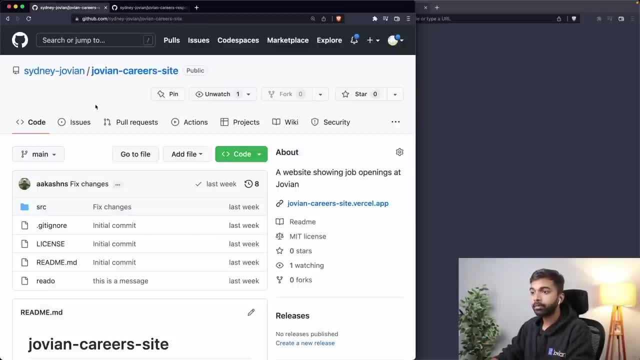 Okay, Now what I want to do is I want to take this GitHub repository and import all the code from this GitHub repository into my new repository. Okay, This is the repository for the previous lesson. I don't want to disturb it Now. normally in a job, you will probably be continuing to work on the same. 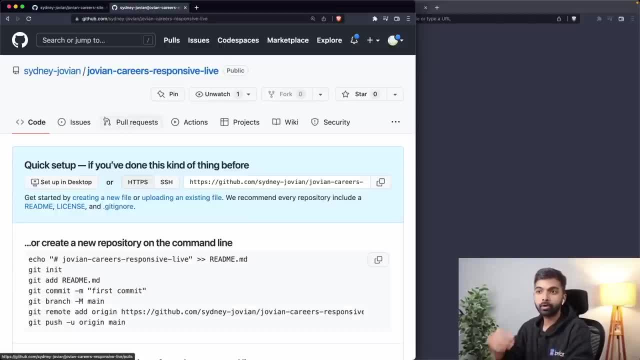 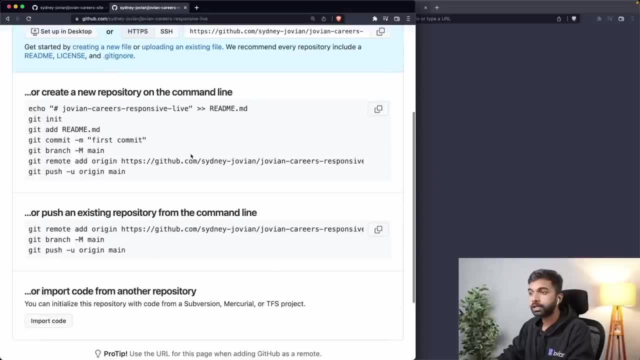 repository, but just for demonstration, I'm showing you how to create a copy so that the previous lesson doesn't get affected. Okay, So there are many ways to add code into a empty repository. You can check out some of these, but here is one called import code. 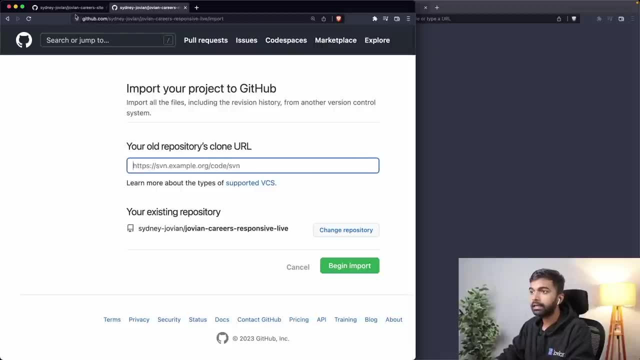 So what you can do here is click on the import code button and then grab the URL of the old repository. So here is the old repository. I'm grabbing the URL Jovian career site and I'm going to copy the code from: or. 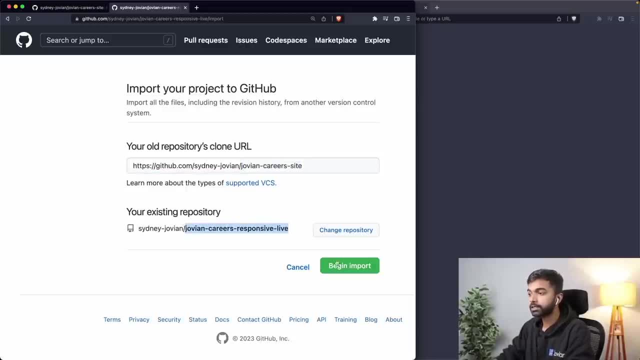 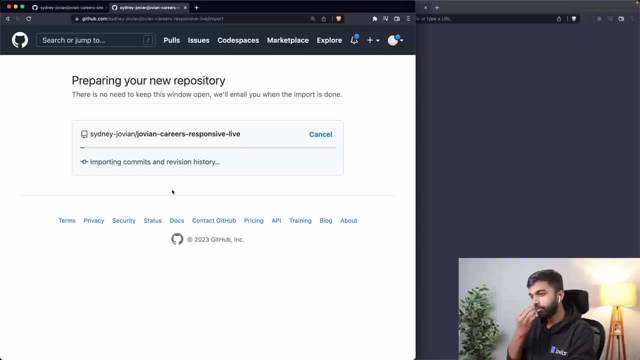 import the code from the old repository into this new repository, Jovian careers, responsive life, and I'm going to click begin import. Okay, Now this is going to take a couple of minutes to maybe import the entire code, depending on how much code you have in your repository. 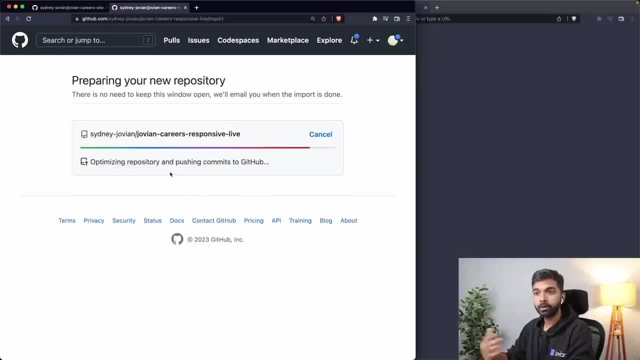 All right, And once we have this, we will be able to now see our new repository and make changes there without affecting the old one. Okay, So our import is now complete, So let's open it up and I can close the old repository. 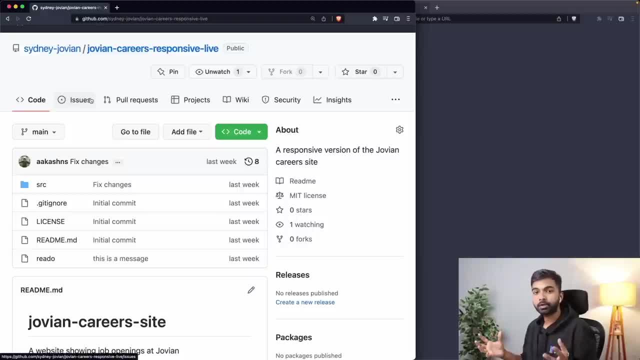 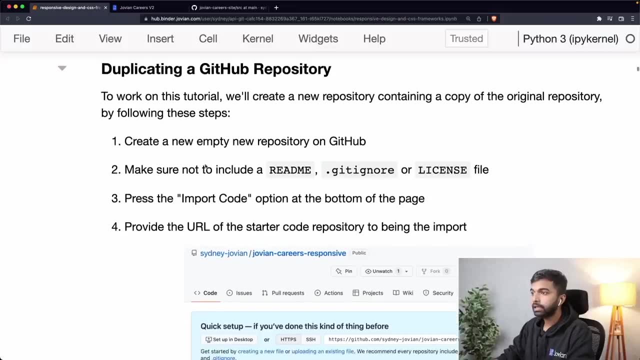 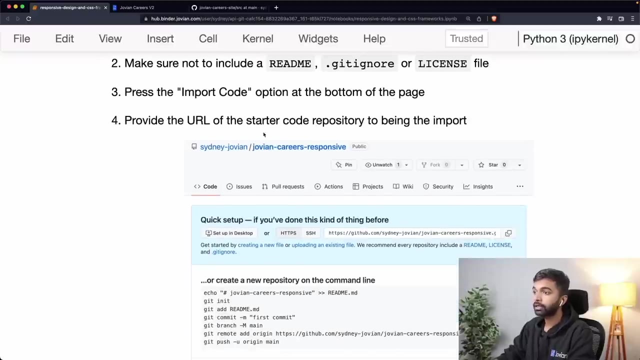 So now I have a new repository with my starter code all in place without affecting the old one. Okay, All right. So that's what we just did. We created a duplicate of a GitHub repository by creating an empty repository, not including a read me: get ignore our license pressing the import code button. 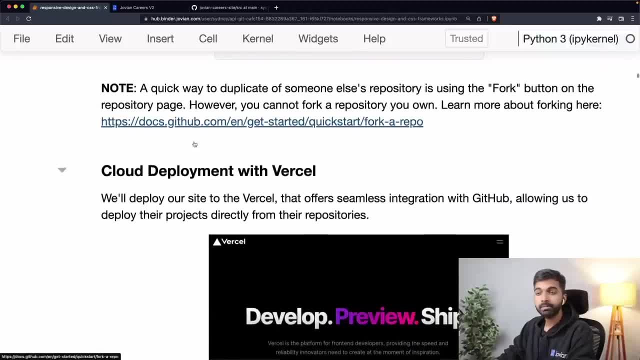 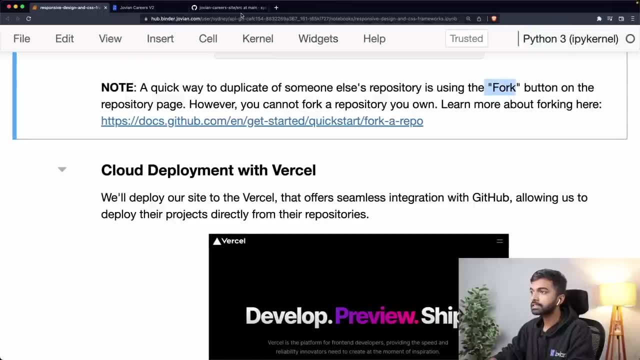 and providing the URL of the starter code. Okay Now, of course, as I mentioned, if you are on somebody else's repository, you can do all of this very quickly using the fork button. So you can see that there is a fork button here, which is disabled for me because 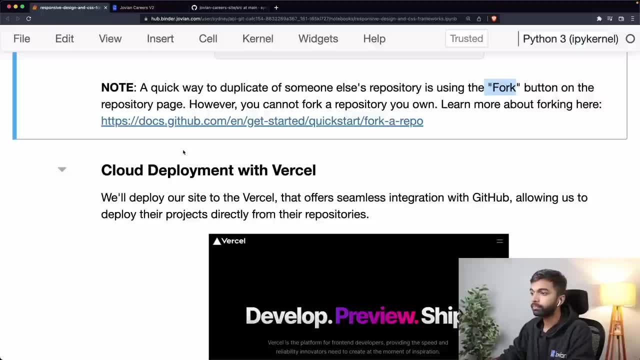 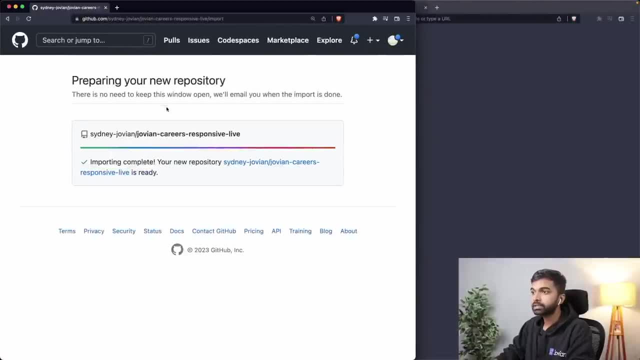 this is my own repository, but will be available for you when you need to. Okay, The next thing we'll do is we will. We will also deploy our new repository to Vercel. So I'm just going to open up Vercelcom and Vercel, as we know, is a deployment. 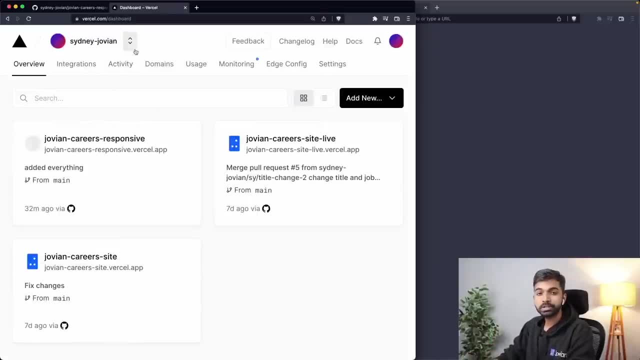 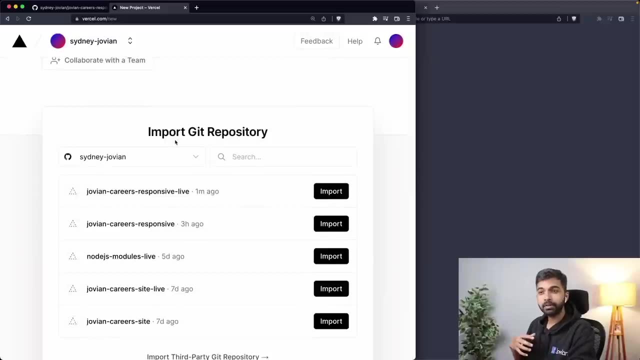 platform that has good integration with GitHub And once you're logged in on Vercel I'm going to add a new project. So I'm going to say add new project And if Vercel is not already connected to my GitHub, then it will ask me permission. 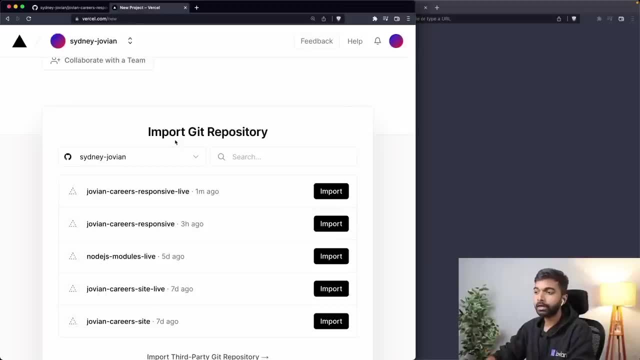 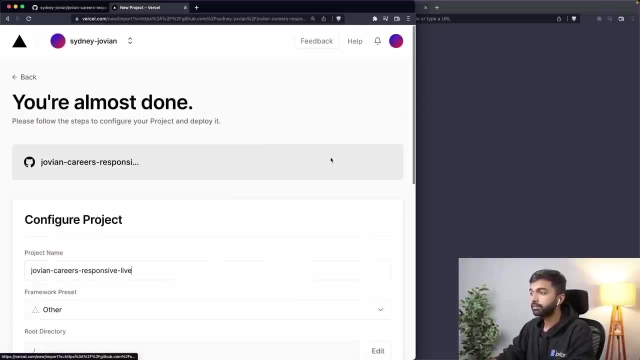 to access my public and private GitHub repositories, which I have already granted. So here I can see. on Vercel I can. I have the option to import the Git repository Jovin careers, responsive life, So let me just go ahead and import that. 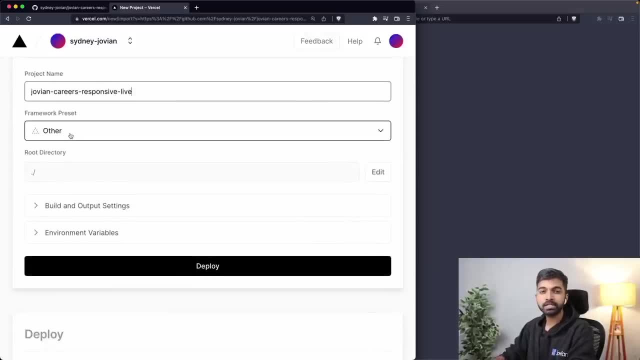 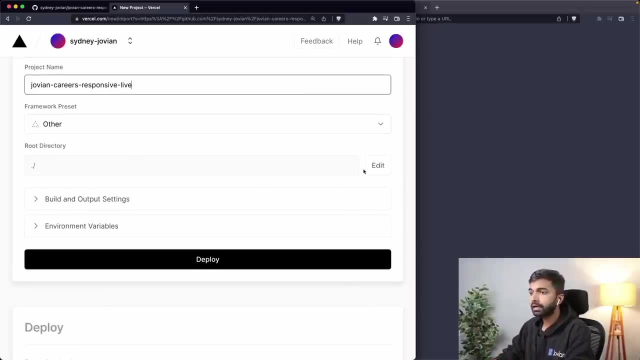 And that is going to create a project and I'm going to use a framework preset other, because I'm not using any framework, It is just a static site with some HTML and CSS, And then I'm just going to click edit and I'm going to go into SRC because I don't 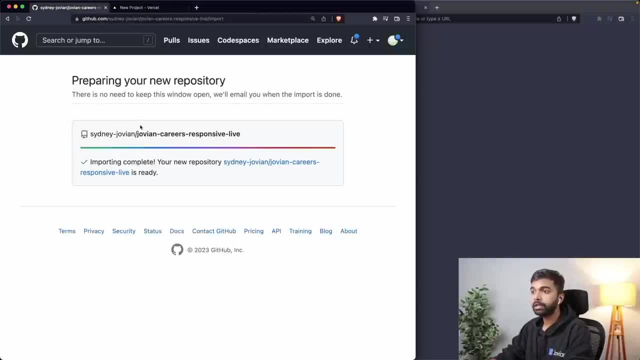 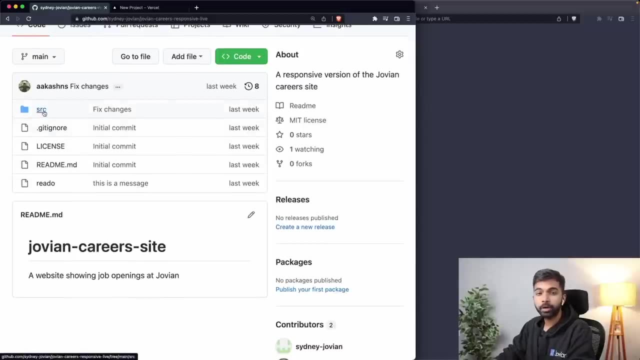 want the entire folder to be deployed. I don't want the entire repository to be deployed, You can see here. I simply want the SRC folder to be deployed, because that is where my index or HTML file or my default webpage is present. Okay, 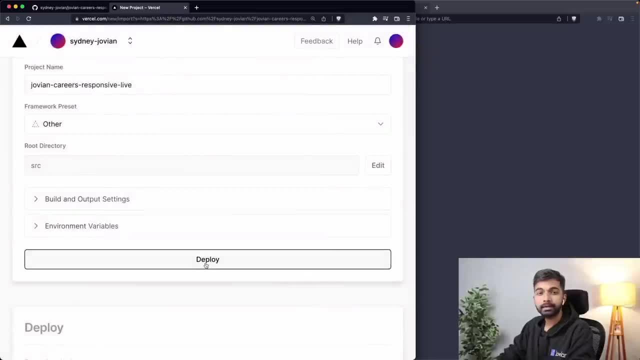 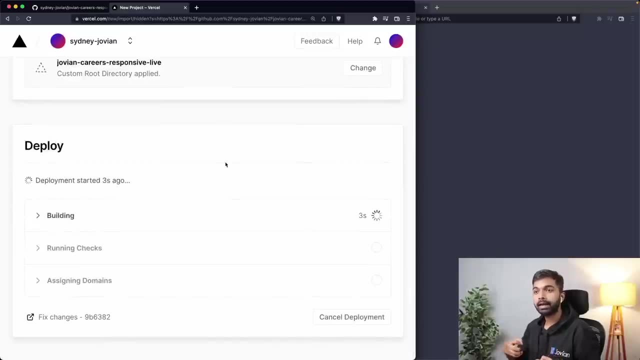 So I'm just going to select the SRC folder and click continue And then I'm going to click deploy And just like that, in just a few seconds that repository will get deployed and I will have my new website Jovian careers live. Jovian careers responsive live. 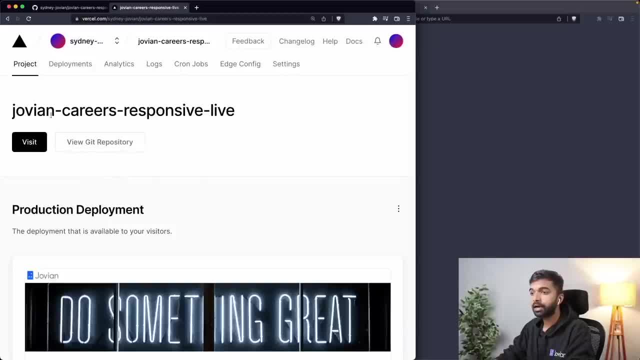 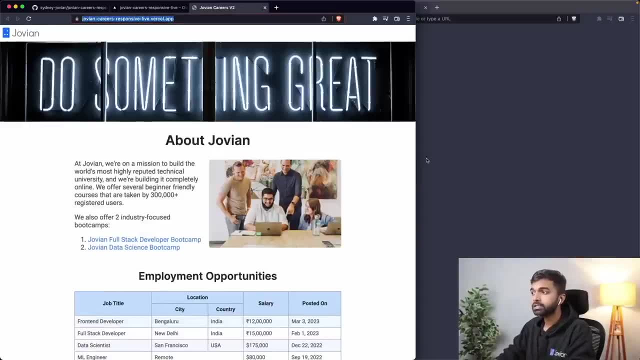 Let me see, I can just continue to dashboard. And now I have my new project, Jovian careers, responsive live dot Vercel dot app. Okay, So now the repository is completely deployed to Vercel and any changes that we make will. 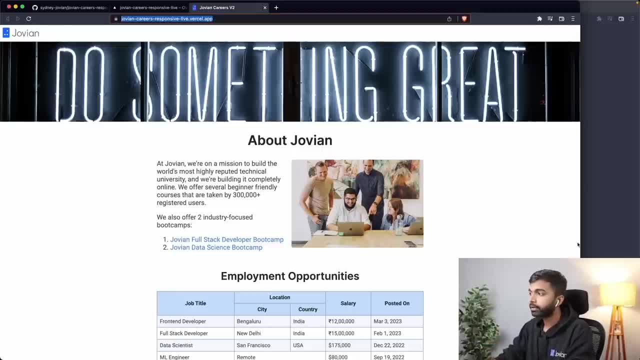 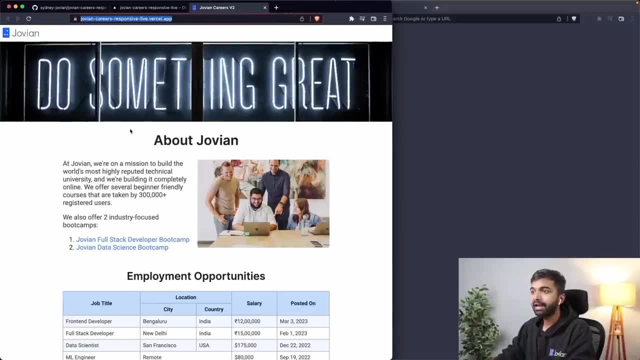 now be affecting this new site. Okay, Perfect, So that's our basic setup in place, So that's good to go. now Let us come back here and also open up the score using GitHub code spaces, so that we can actually start writing some. 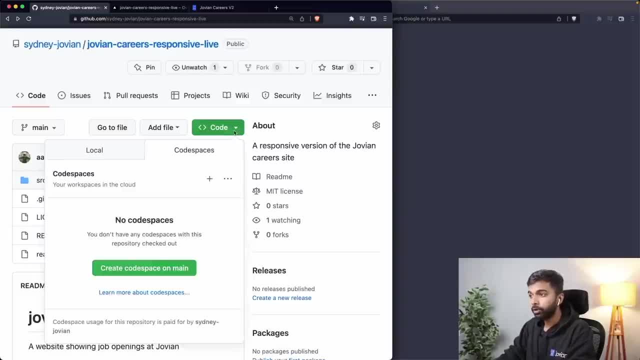 code and start editing things. I'm going to click on code and here now I can create a new code space on main. And remember, a code space is a local machine for us on the cloud, given by GitHub associated with this repository, And we'll be able to write our code in that code spaces machine. 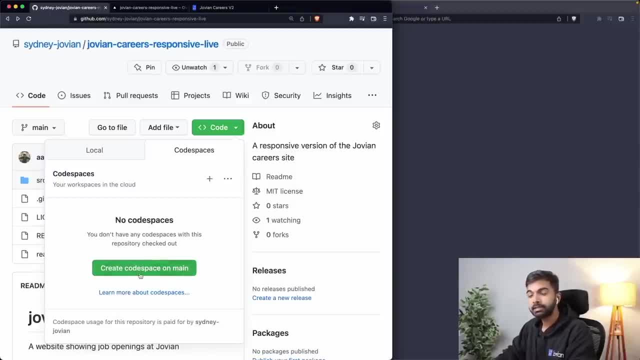 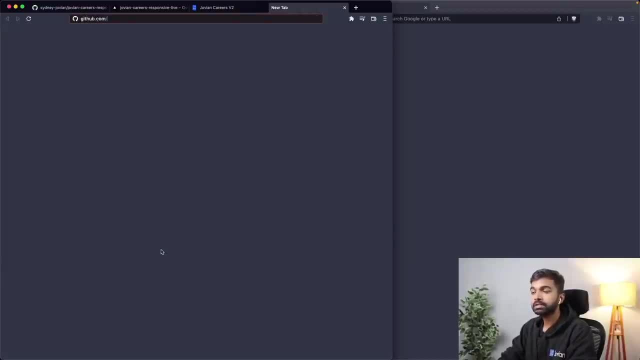 So let's click create code space on main And, by the way, if this button is disabled you may have to go ahead and delete some older code space. So you can go to githubcom slash code spaces, And I think GitHub provides two code spaces for free. 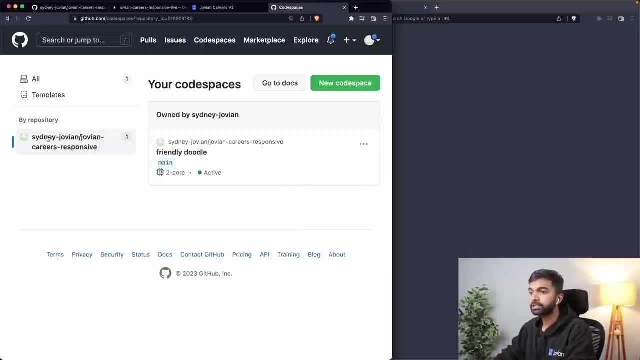 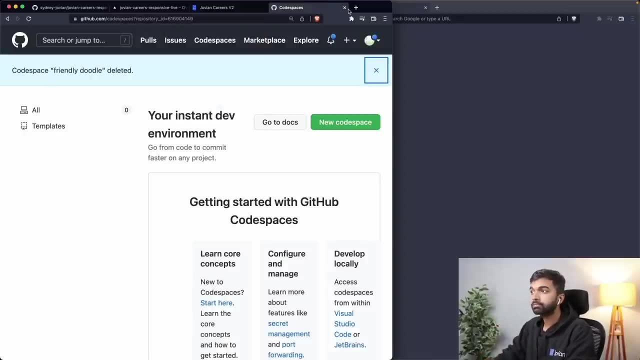 So you may have to go in and maybe delete an older code space. So you can just go to an older code space and click delete, and that's going to delete your old code space, so that you can now reload this page and actually access this button. 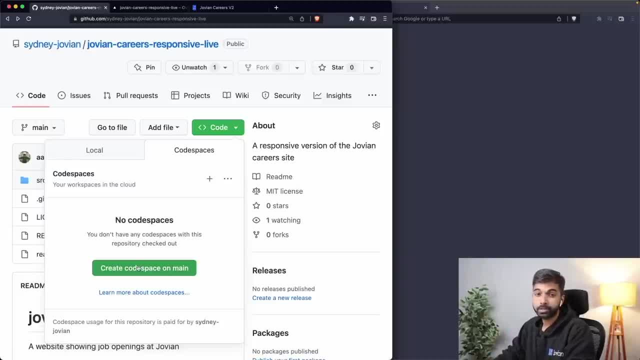 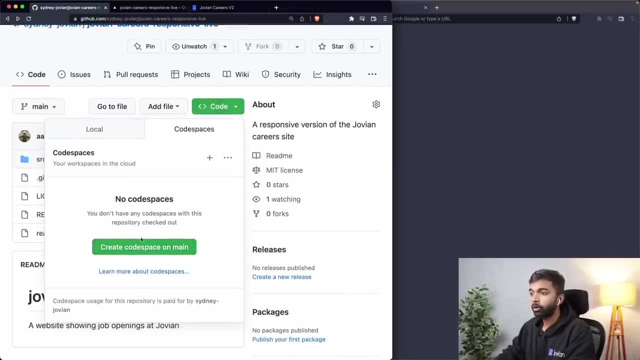 Okay, So you can have only two free code spaces. Otherwise you can pay and you can get unlimited number of them, but free should be fine. You can just delete Code spaces when you need. Okay, So let's click code and then let us click create code space on main. 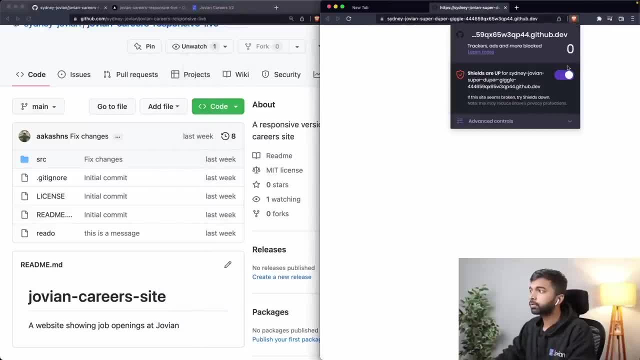 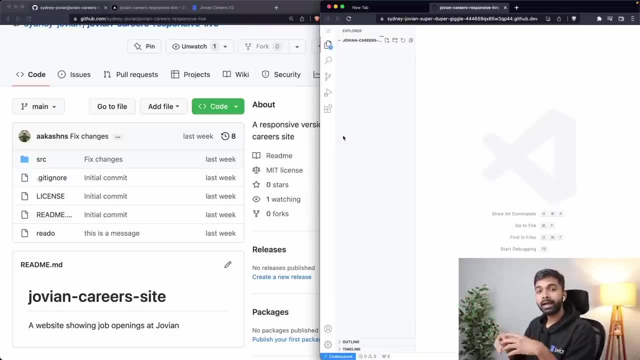 And let me bring this over here Now. what this is going to do is open up a machine on the cloud, get the code from the repository and give me a browser based interface of visual studio code to edit and test and develop the code from this repository. 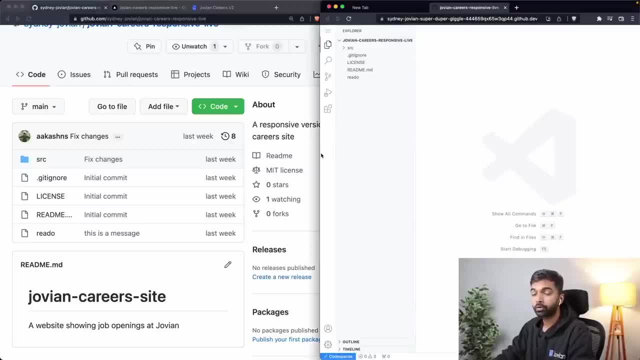 Okay, So GitHub is for storing the code, visual studio code Code spaces is for actually developing the code, and then I can take my changes and push them back either onto the main branch or I can use the GitHub collaboration workflow where I can create a pull request and get that reviewed, and so on. 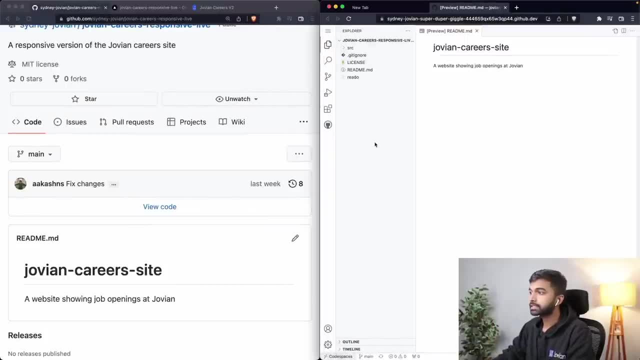 Okay, All right. So it looks like our code spaces system is now open and ready for development, So I'm just zooming it in a little bit, but you can see that this is a visual studio code interface, and let me just close that. 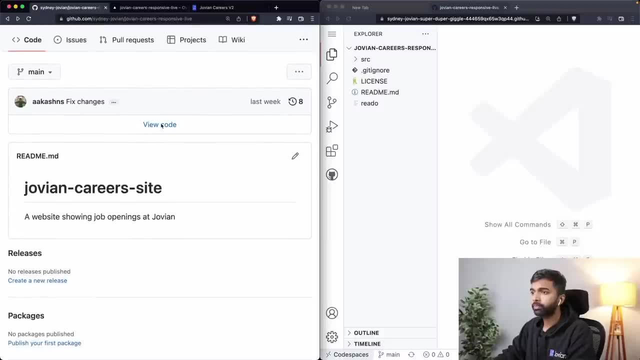 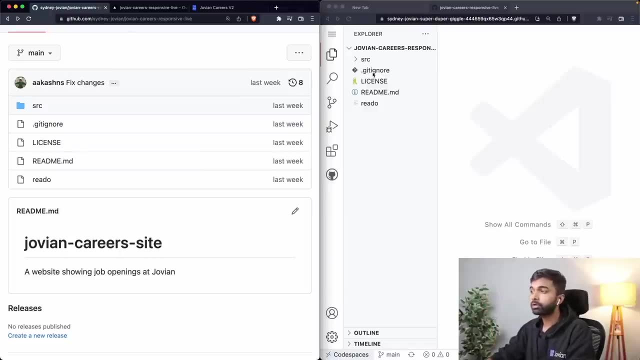 Now, here we already have the repository, the root file of the repository, open. You can see that we have an SRC folder. We have get ignore license. Read me: all of these are imported in from the original repository. I can open up the SRC folder and open indexhtml. 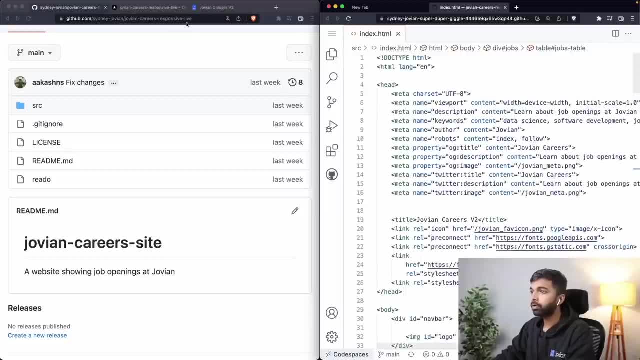 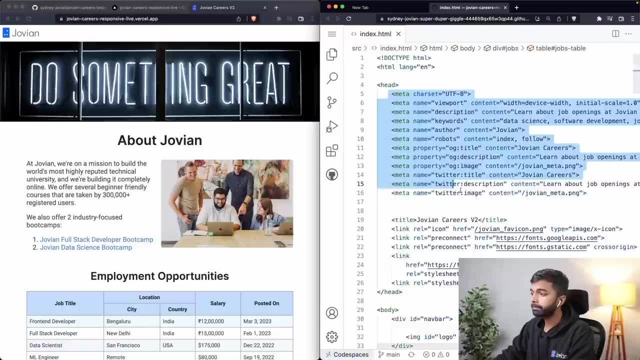 And here in the indexhtml file I can see the entire code or my website, Jovian couriers. So you can see that we have a head, We have an HTML tag inside which we have a head tag in the head tag. 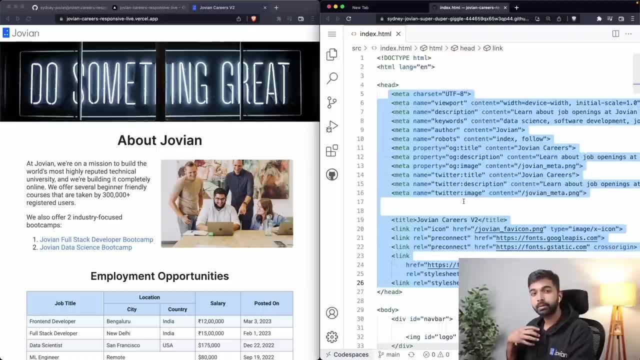 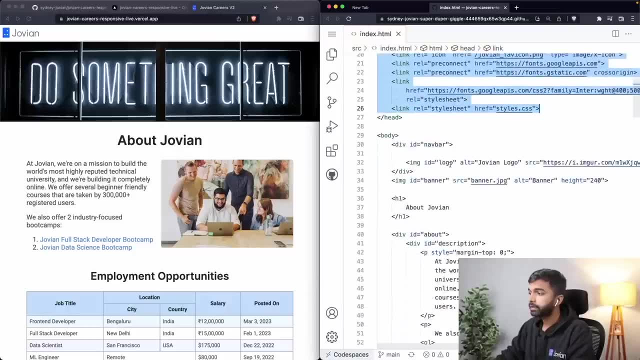 We have a bunch of meta tags to set How this page previews when we share it online. We also set, for example, the title and the fav icon of the page. Then we have the body tag and in the body we have the nav bar. 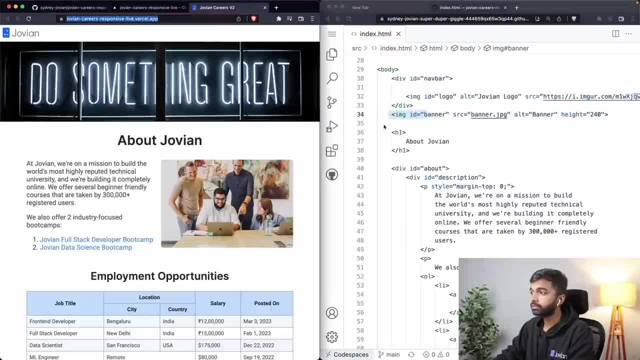 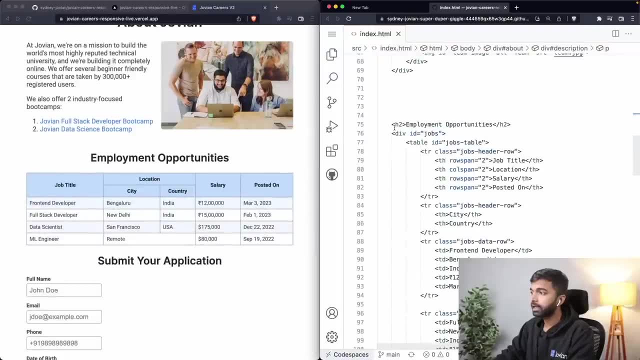 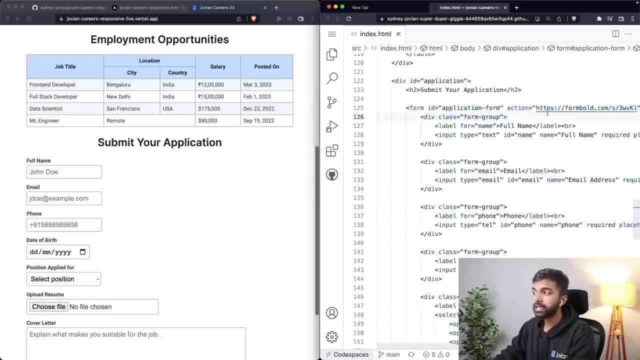 And this is the nav bar. We have a banner image. This is the banner image. We have a header, We have an about section with an image and some description. Then we have a table here The table contains the employment opportunities. Then we have some a form here, an HTML form, and that form makes us 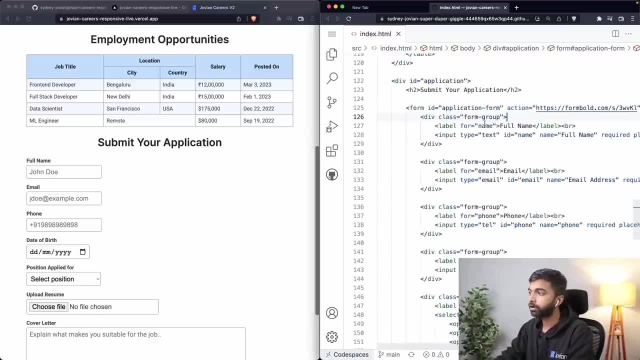 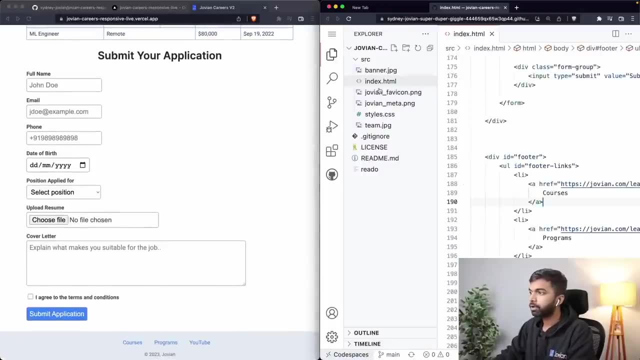 Submission to form bold, which is an external service that we're using for form submissions, And finally, we have a footer here, which is the footer right over here. Okay, And of course, we have all of the styles here captured in stylescss. 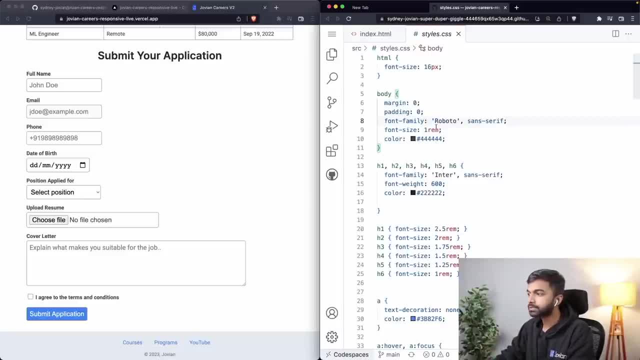 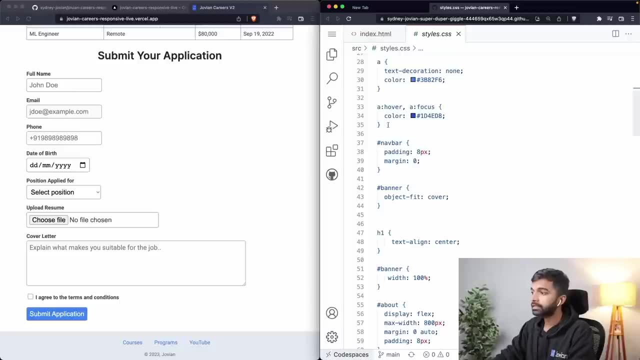 So each section has it. it has its own various set of styles, which is what we've captured in stylescss. So there are some basic styles for HTML body H1,, H2,, et cetera, And then there are section wise styles for each section and then the subsections. 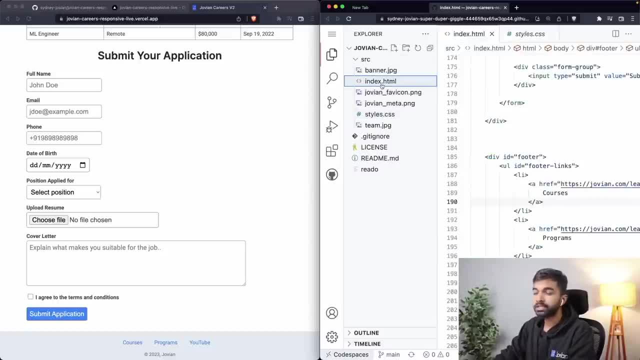 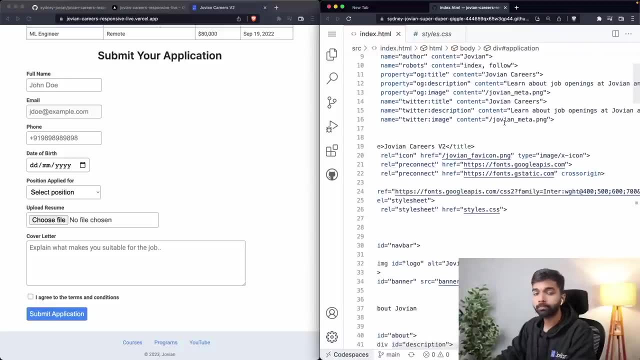 inside those section, and so on. Okay, And we have certain images as well which we are incorporating within the page, And, of course, we have- uh, we are connecting the styles with the main page using the link here, the link rel equal to style sheet. 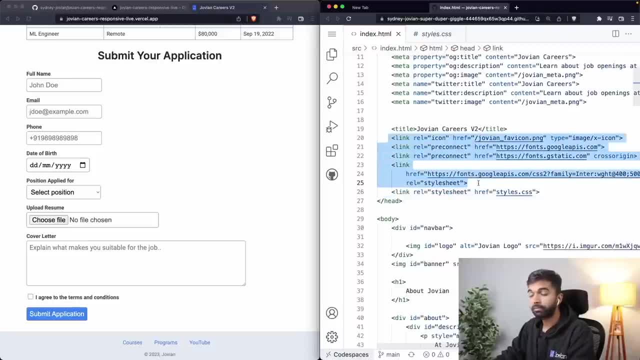 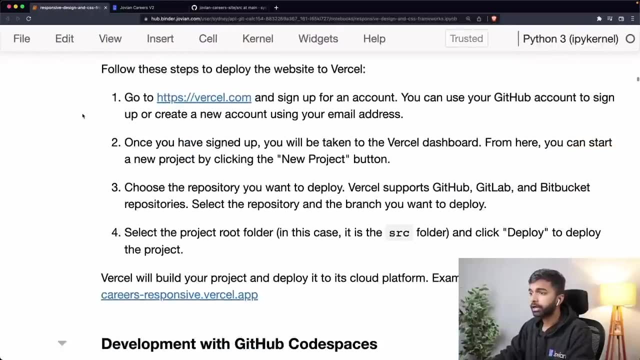 Plus, we're also using some external fonts from Google APIs, uh, from, uh, Google fonts. Okay, So this is a basic setup that we've explored so far. All right, So now we've looked at how to deploy to the cloud using Vercel. we've looked at how to. 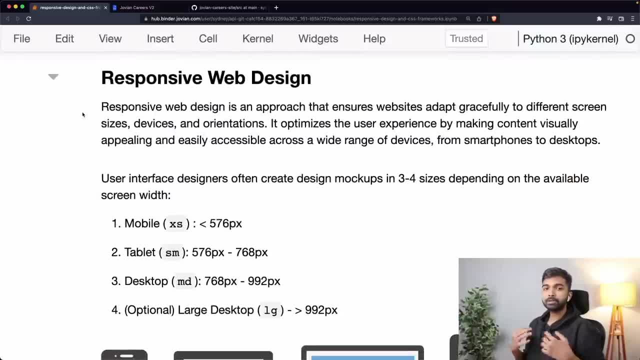 start development with GitHub Codespaces. now let's talk a little bit about responsive web design. Responsive design is an approach that ensures that websites adapt gracefully to any screen size, any device and any orientation, And that is the purpose. here is basically to optimize the user experience by making 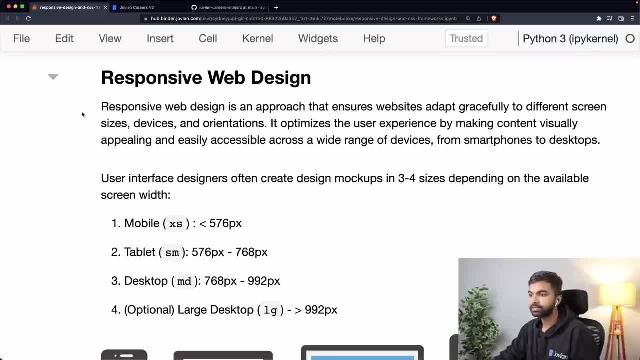 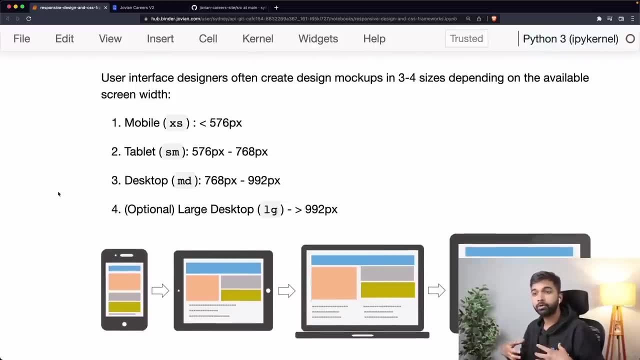 the content visually appealing and easily readable and accessible. Okay Now responsive design starts from the user interface design. So even before you have started coding the page, user interface designers will often create design mockups in three to four sizes, depending on the available screen width. 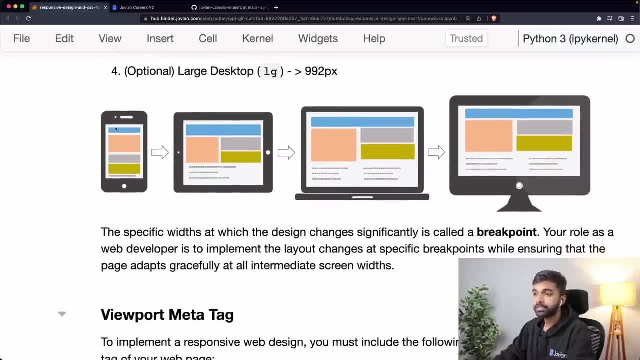 So they will create a mobile design. So let's say they're designing a website. They will first create a mobile design and in the mobile design everything just goes top to bottom. You generally don't don't have a lot of things side by side because the limit 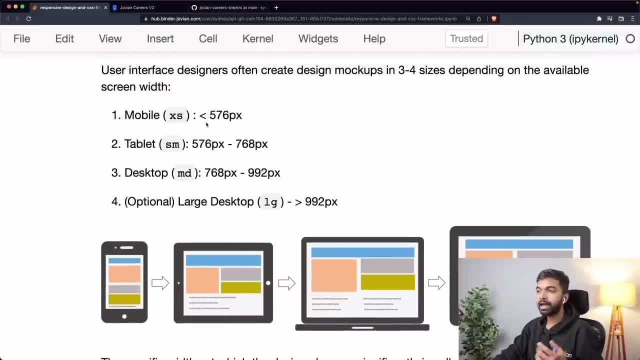 On the, because the screen width is very limited And, in fact, just as a common practice, something around 576 pixels and below is considered a mobile screen, just for reference. So typically you will get a mobile design which is about, which is. 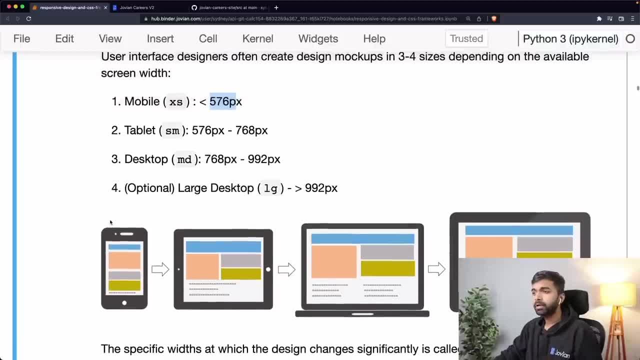 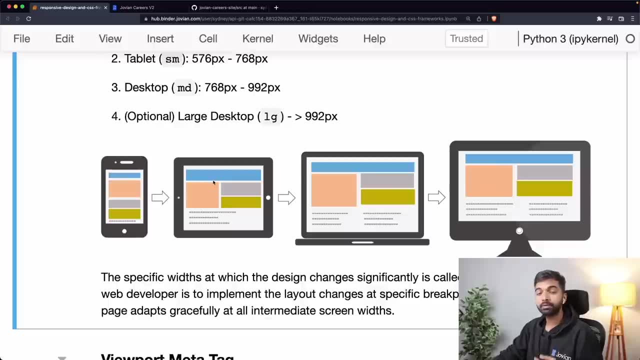 something under 576 pixels in weight, Then they will often give you a tablet design. Now the tablet design will have maybe two columns in certain places. in certain places There will still have one column. So certain things you have slightly more space horizontally on a tablet. 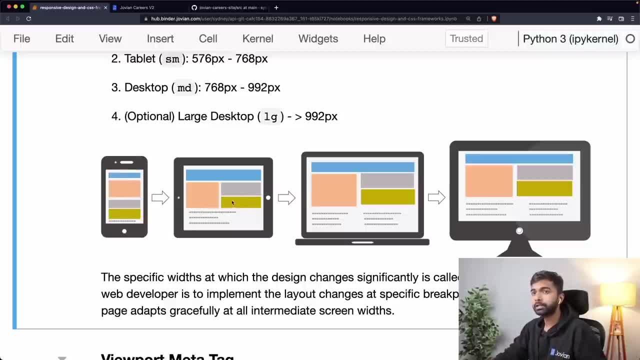 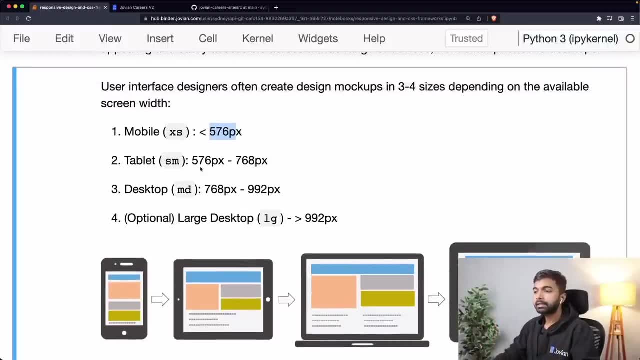 And that's why there might be a slight change. You can see that these two sections were brought in here on the side on a tablet screen, And typically tablet screens are about five T to seven, 50 pixels, And then you have desktop screens. 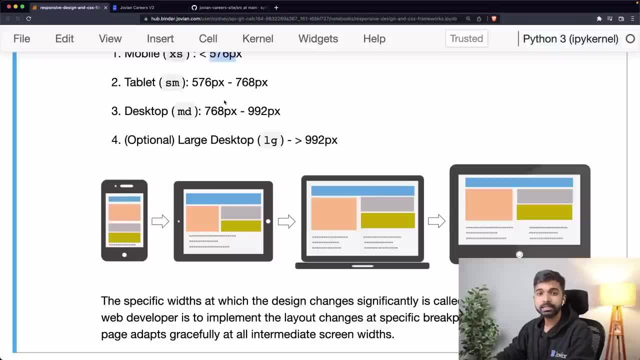 Desktop screens are screens that are bigger than seven- 68 pixels. So this is where you have a lot more space. This is where maybe you can use three columns, This is where maybe you can have more space on the left and right And finally, optionally, sometimes you will find a layout for large desktops. 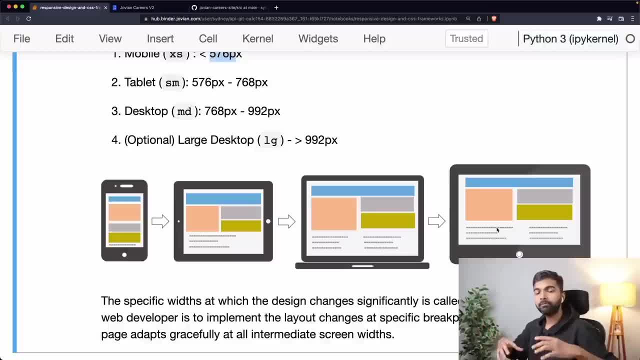 So often now as we are getting to bigger and bigger screens, like four K screens and eight K screens and so on, we have the opportunity to use a lot of, Leave a lot of blank space on the left and right. So sometimes, especially if your website is going to be viewed by people primarily on the desktop, 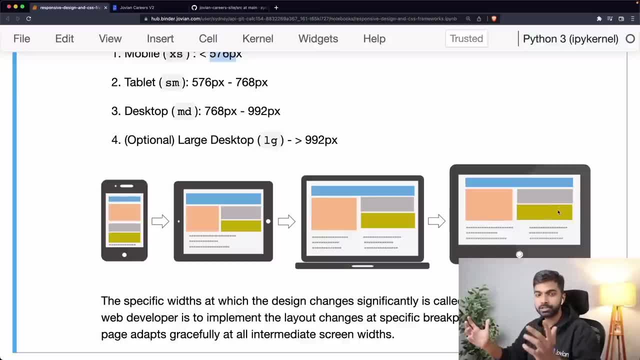 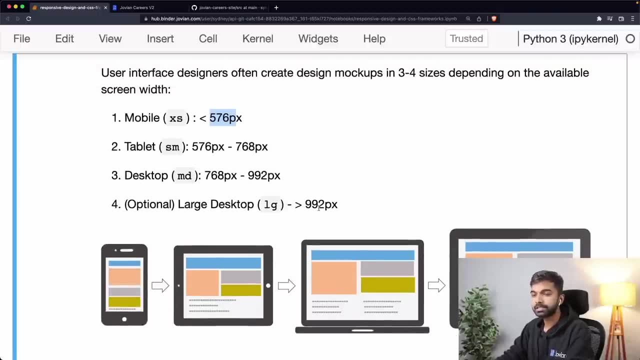 you may get a fourth mock-up or a fourth design or very large desktops. Okay, And typically this refers to a desktops with a screen width of greater than 992 pixels. If you don't get a design like this, then you should just take the hint that you should take the desktop. 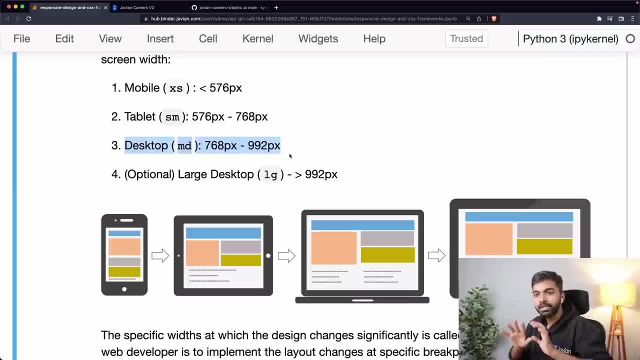 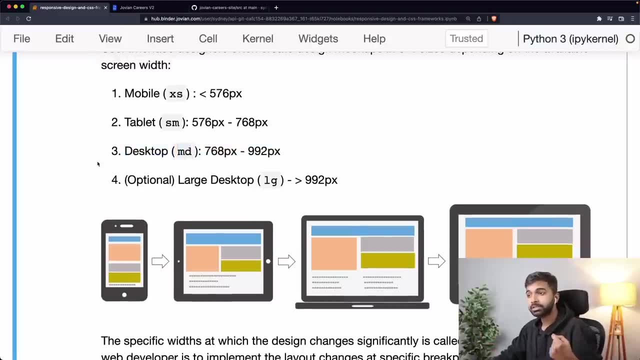 layout and just limit its width so that the content remains centered on the page instead of completely spreading left To right, making it hard to read. Okay, So your designer will often give you three separate layouts at least, and sometimes even four, or sometimes you may just get two. 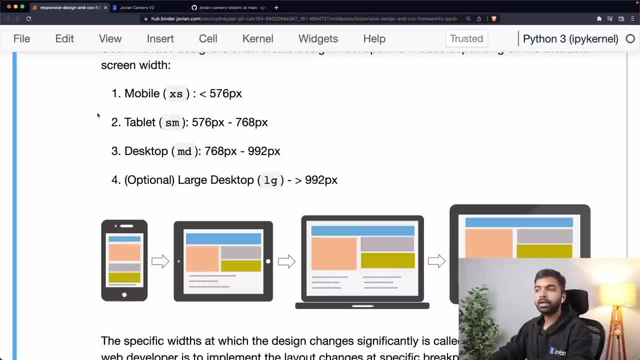 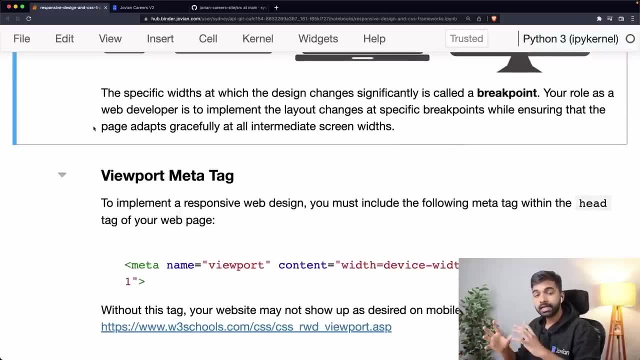 layouts, one for mobile and one for desktop, And you may have to guess what the tablet layout looks like. Okay, Now the specific weight set which these design changes are made, where the design changes significantly are called break points, because the previous design breaks at the at that point and a new design takes over from there. 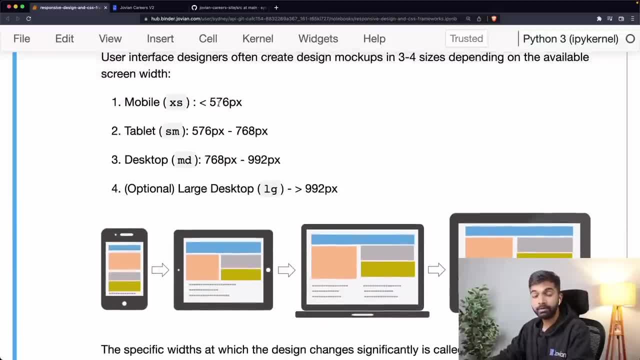 Okay. So the break point for mobile Okay Screen is 576 pixels. beyond that It's the tablet screen. And then the break point for desktop screens is at seven, 68 pixels. beyond that It is uh. beyond that it is a large, beyond that it is a desktop screen. 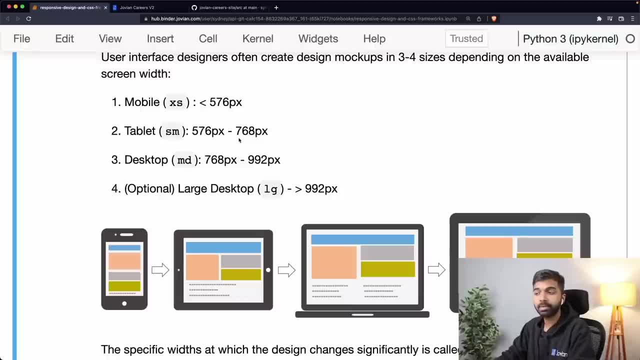 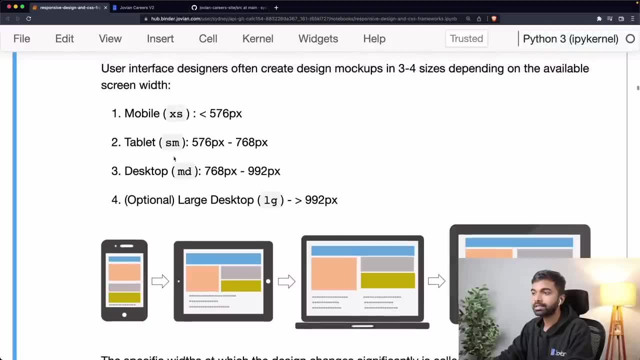 So the break point or the highest break point for tablet screens is seven- 68 pixels, And beyond that it is a desktop screen, And then sometimes beyond 900 pixels or so it is a large desktop screens. Now, these numbers are not set in stone. 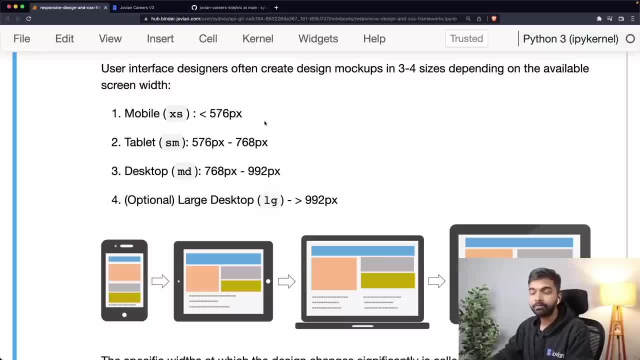 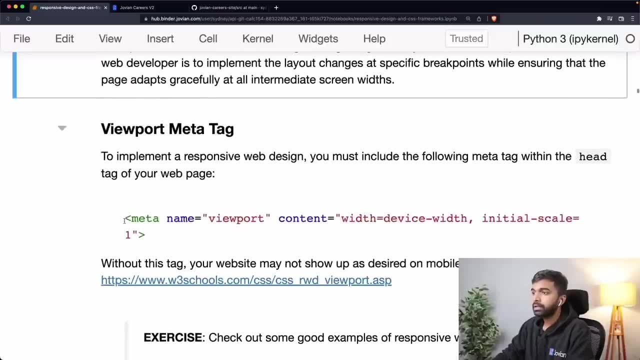 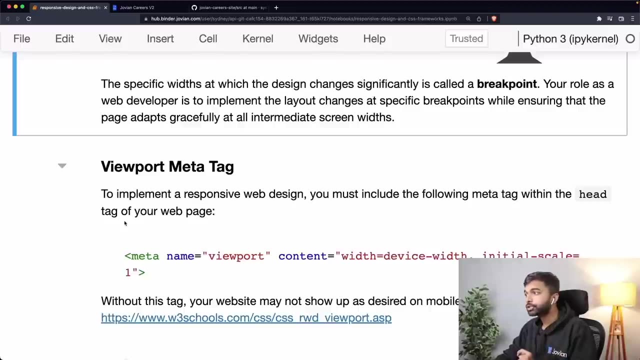 These are just Some common values, but different sites, different frameworks that we use for CSS, have different values, but these are just some of the more standard ones. Okay, Now your role as a web developer is to implement layout changes at specific break points, while ensuring that the page adapts. 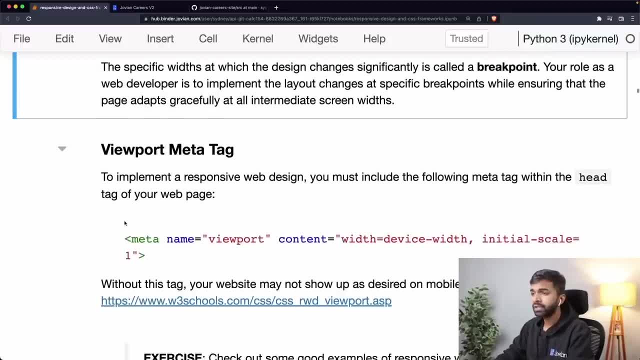 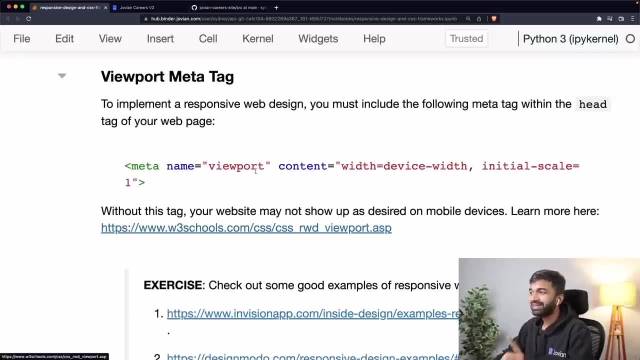 gracefully at all intermediate screen rates. Okay, And that is what we're going to learn today. Now, one important thing to keep in mind whenever you're trying to make a website responsive Is that to make a, to implement a responsive web design, you must include this following meta tag within the head tag of your web page: 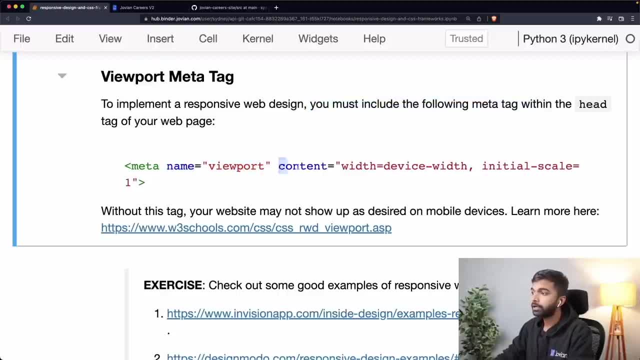 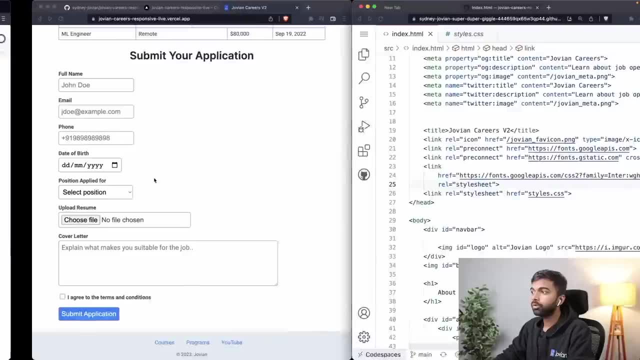 So this: there's this meta tag with the name viewport and it has a content with device width and initial scale equal to one, or sometimes this is written as 1.0, and you have to take this and you have to put this inside the HTML head tag of your HTML page. 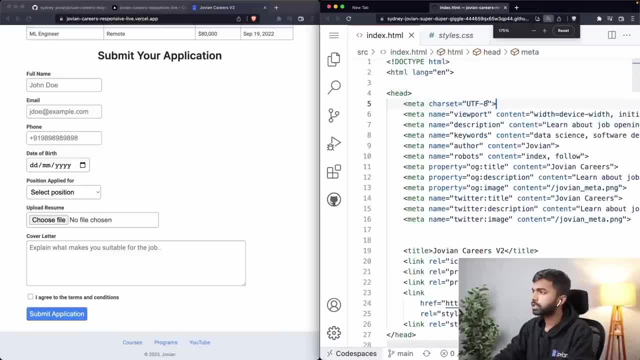 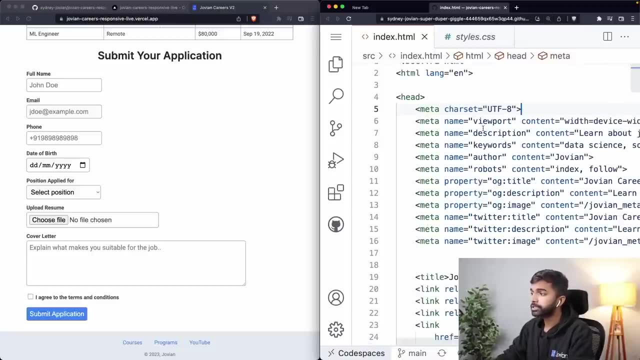 Okay Now in this case I already have it- meta viewport. Let me zoom in here slightly. Yeah, you can see here I have the tag meta viewport with device width, initial scale 1.0.. Why is this important? 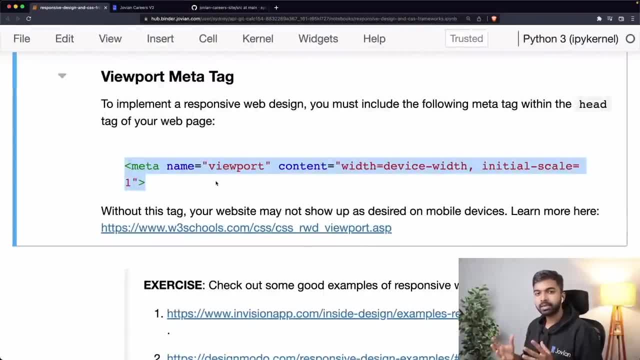 Well, back when mobile mobile smartphones just came out, there were no designs that were optimized for mobile screens, So there were certain tricks that were employed by mobile devices to zoom in and somehow scale and make the text more visible. Nowadays, those tricks are no longer required because developers implement responsive designs. 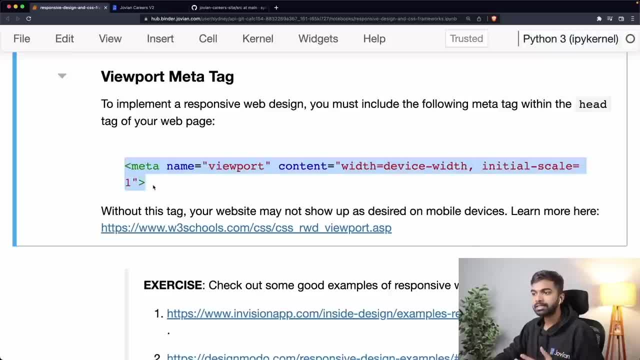 So that's why Indicate to your browser to indicate to the device that please don't apply any tricks to make the content look good on mobile. I will handle it myself. You include this meta tag. So all you need to know is, whenever you're making a design responsive, make sure that you have this meta tag included in your design. 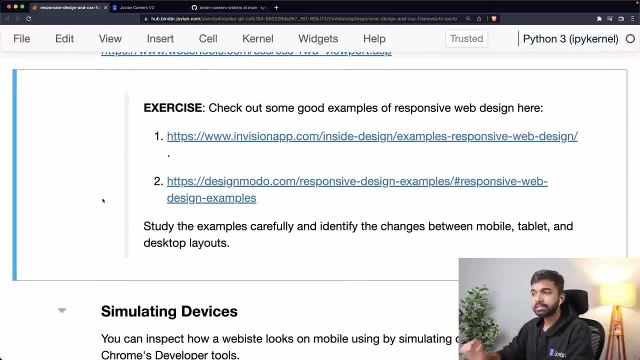 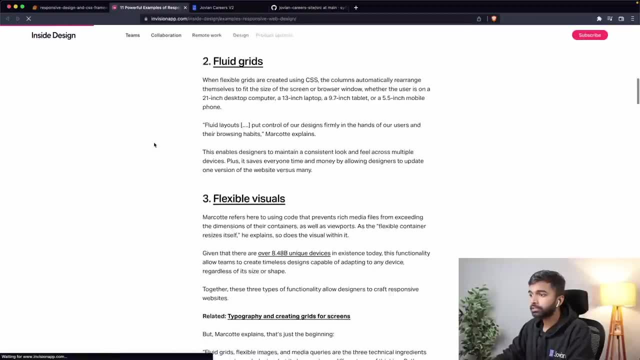 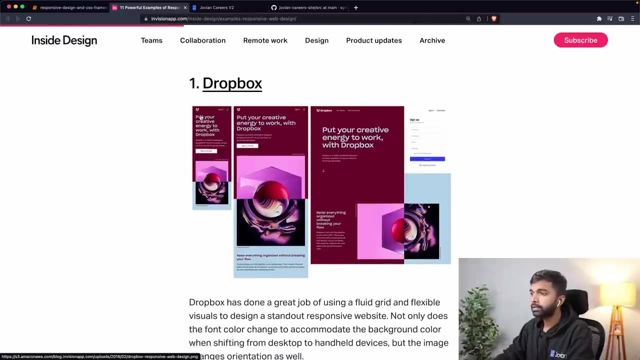 So one good way to build your responsive design skills is just by checking out some examples of response to design. So here's one. you can check out a bunch of examples here. So here is one. Dropbox, The homepage for Dropbox is a good example, where this is the mobile view. 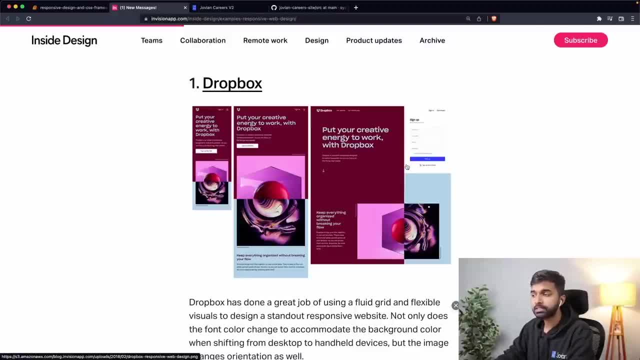 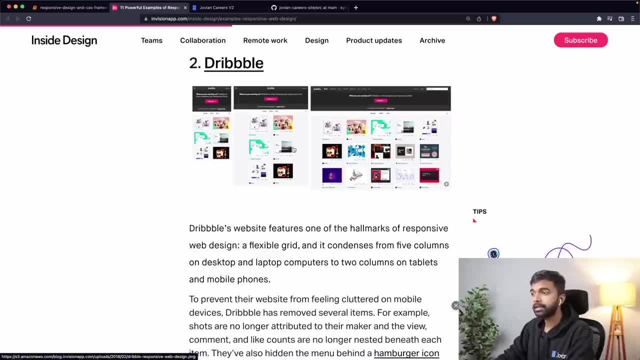 This is the tablet view And this is the desktop view, which also contains a form It was. here's another one. This is dribble, It shows images. So here you can see that on mobile it shows two images side by side on desktop. 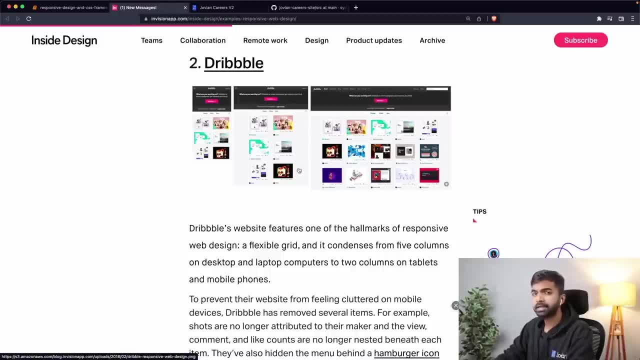 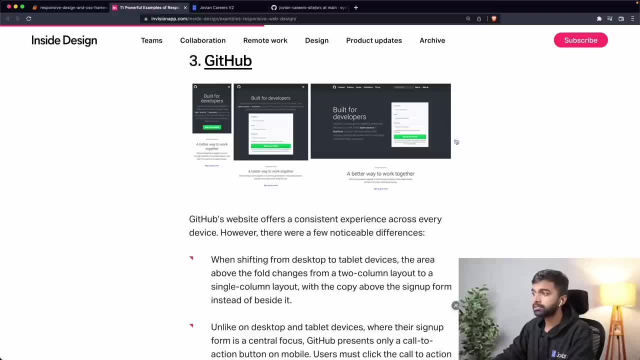 It shows four, five images side by side and then a tablet. It's somewhere in between. GitHub is another example that there is often you will find this pattern that in the desktop layout there is Space on the left and right. There is possibly a form in somewhere on the right. 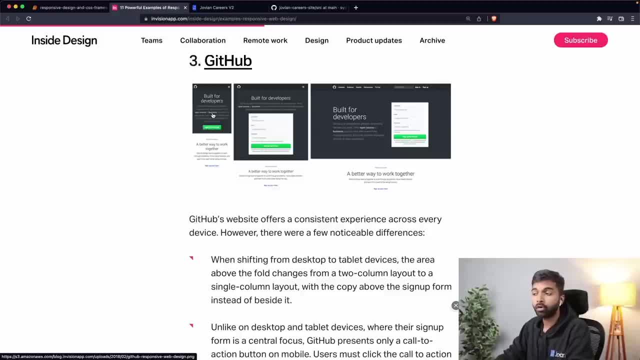 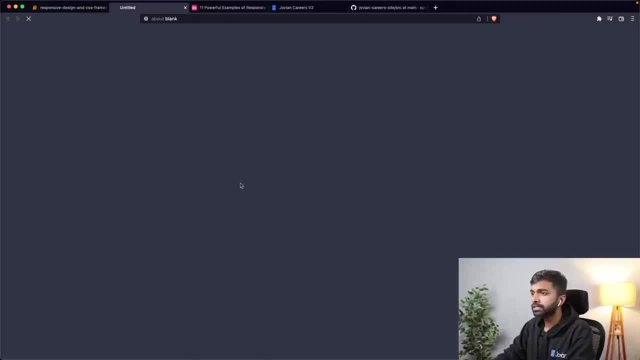 And then in tablet the form comes in the center, and on mobile the form can go away altogether, And there are a bunch of other examples that you can check out as well. Similarly, there are again some more examples here for you to check out. 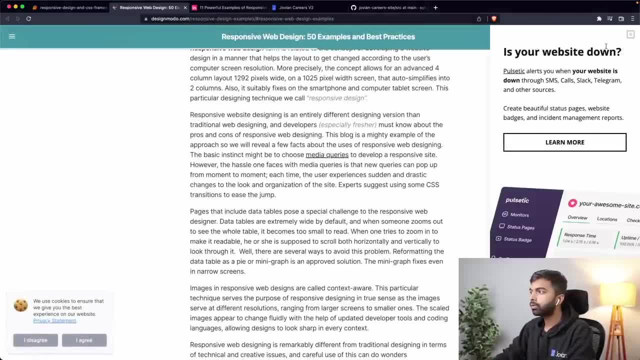 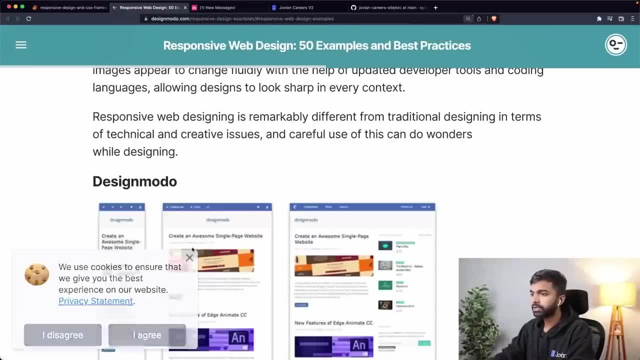 So whenever you're trying to make your website responsive, it's useful to look at how other websites are doing it. You can see your examples of design model So they have this layout for mobile, tablet And desktop. you can see this architecture site. 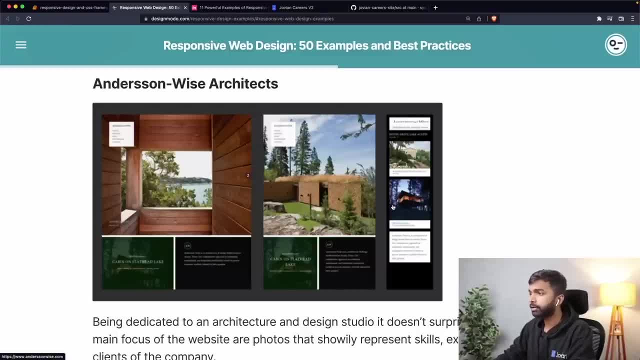 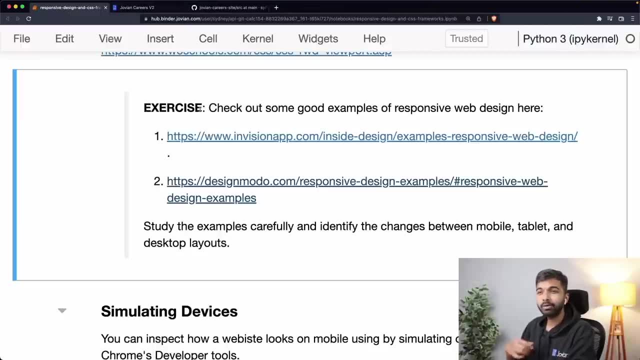 They have a different layout for desktop, tablet and mobile. and here's another one. This seems to be like a personal website. So to become a good web developer, you have to go and explore what other people are doing. There are no ground rules. 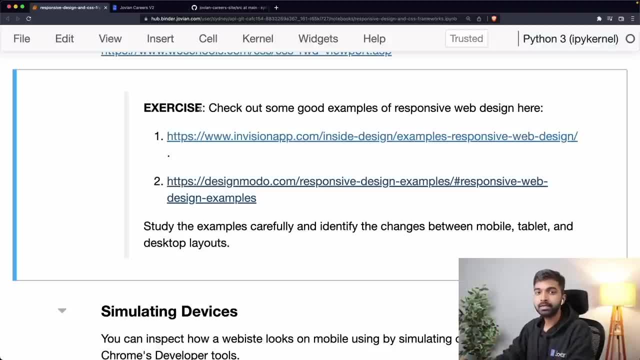 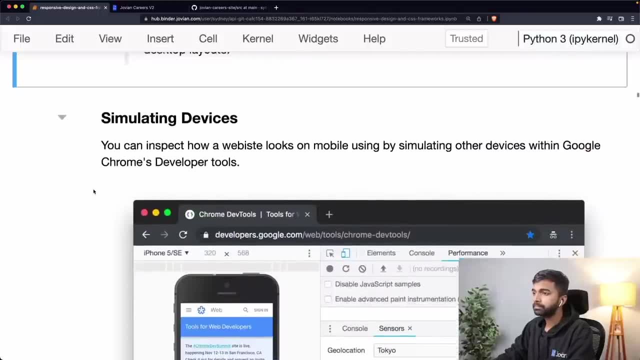 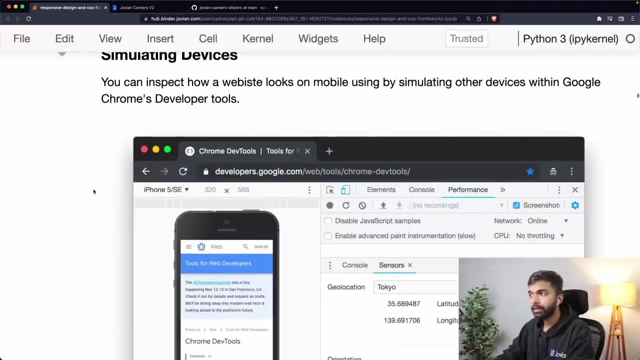 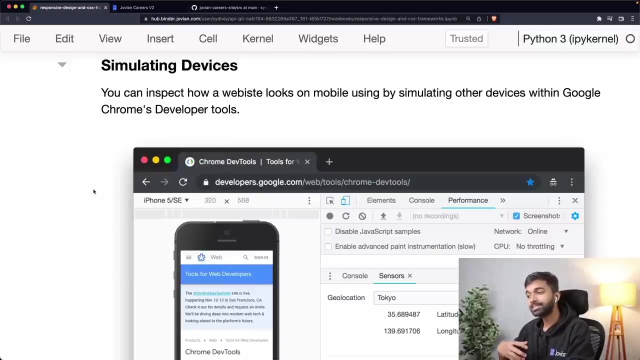 There are no set rules for responsive design. In fact, these trends are constantly emerging, So just explore and pick whatever you feel is working well. Now, how do you Develop a responsive websites So you can inspect how a website looks on mobile by simulating other devices within your browser's developer tools, so that you don't actually have to go and open that website on your mobile each time you want to test it? 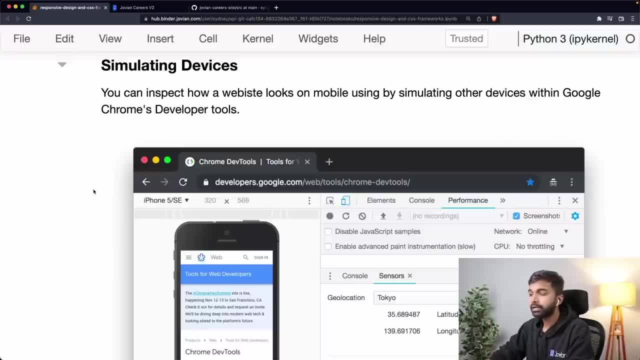 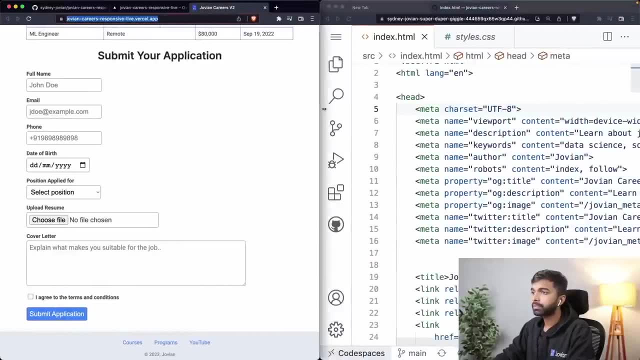 That's a good idea. You should always do a final device test, but you can just do that within your browser itself. Let me show you an example. Let us open up this. Let us open up this job and career site And let me just zoom back. 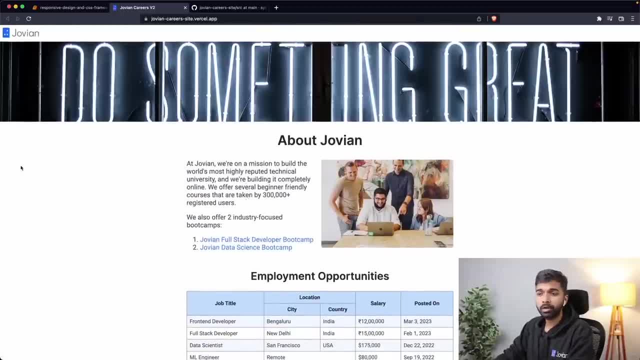 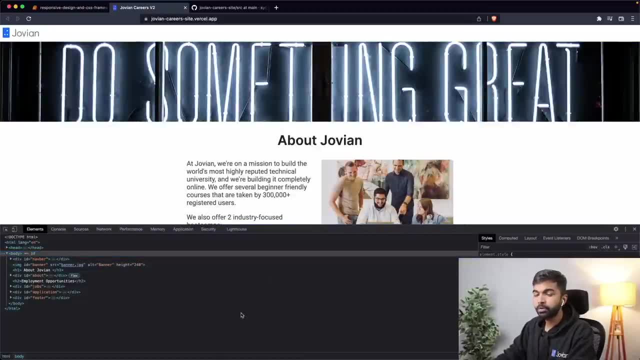 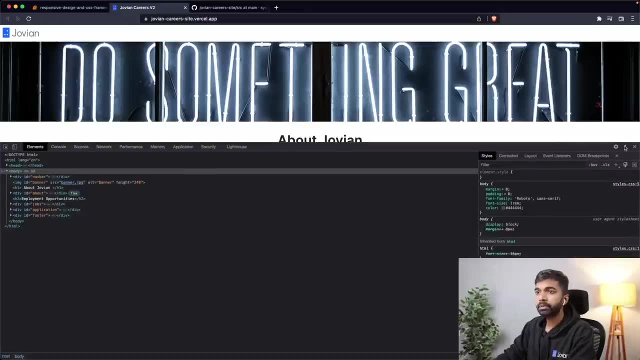 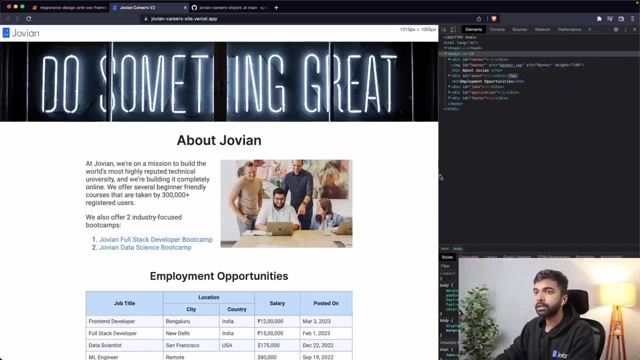 200%. So this is what the career site looks like on desktop. If I right click and I select inspect, now that opener opens up these developer tools and I can just put these developer tools on the right. So there's this button here on the owner, this three dots button, and I just click this three dot button and dock the developer tools to the right is now my developer tools are on the right side. 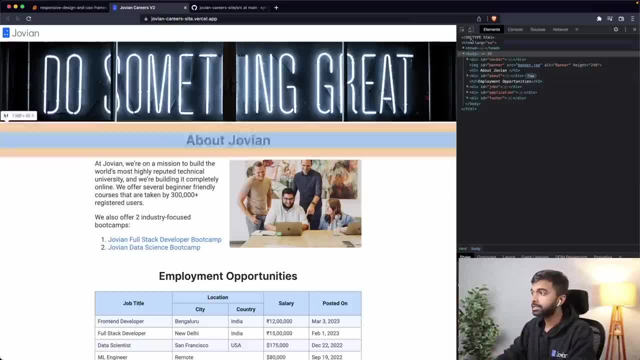 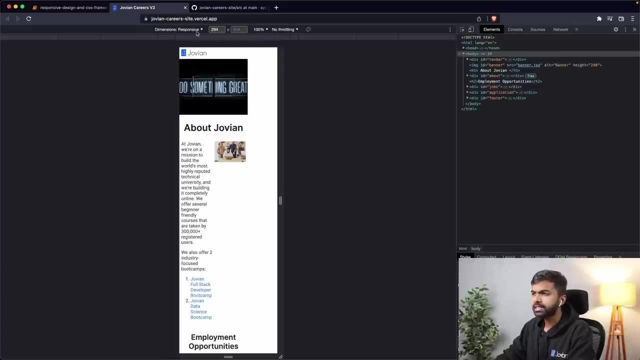 It's exactly the same, but I'll show you in a second Why. putting it on the right head. And now there is this button over here and I'll just zoom in and show you. So this button is called toggle device toolbar. So if you just press this button now, suddenly your browser turns into a mobile device and you can go in and select a specific device as well. 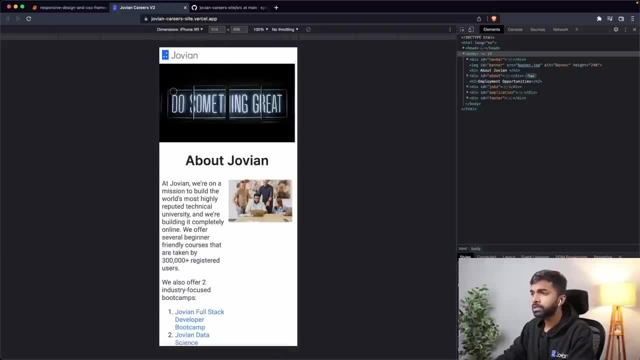 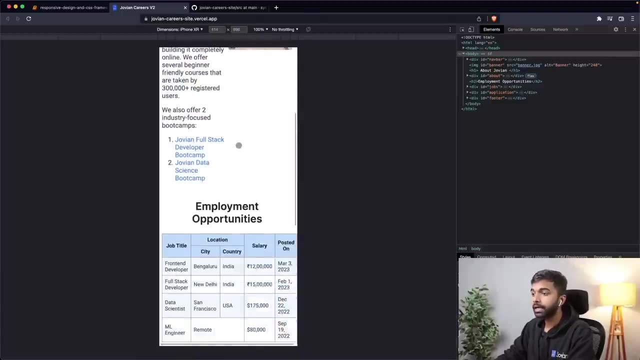 Let's say, let me select iPhone 10 R. So this is iPhone 10 R and this is what my mobile and this is what my and this is what my website is going to look like on iPhone 10 R. Okay, 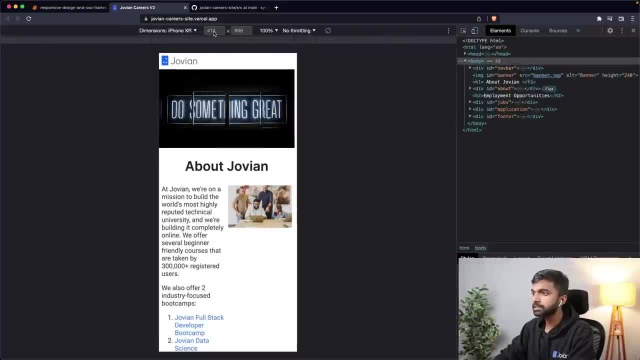 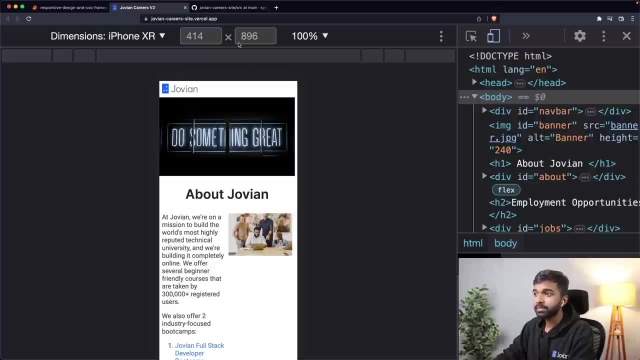 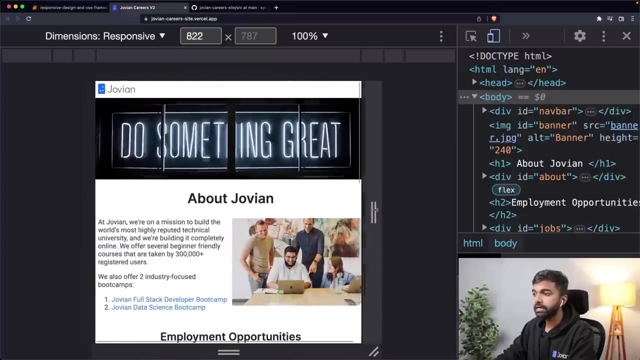 I can even check That the screen width here is 414 pixels. Let me just zoom in there a little bit. So the screen width here is 414 pixels. So that tells me that this is an iPhone 10 R, or I can even just select the option responsive and I can just vary the width of the screen and see how my website changes. 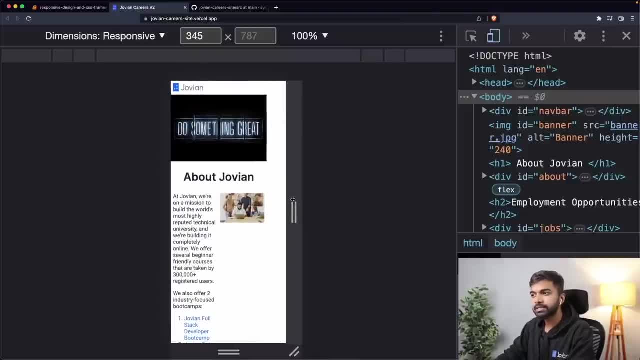 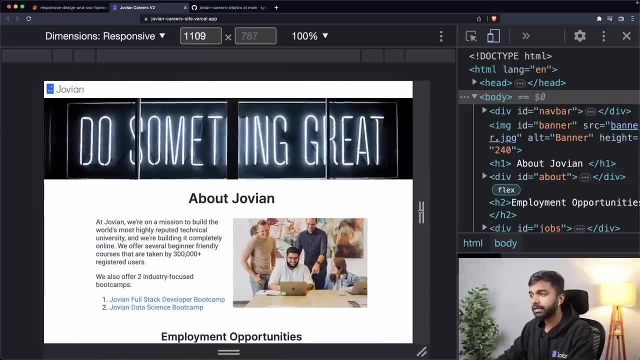 And normally you will not be viewing a website on under 360 pixels, So normally you might want to start around 360 pixels and just vary the width of your screen slightly And see how the website looks as you increase the width. Okay, So this is a great idea. 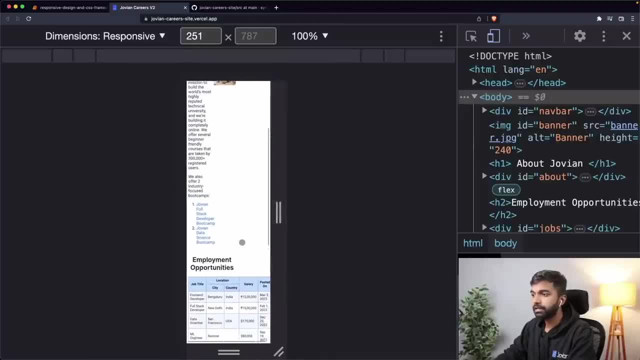 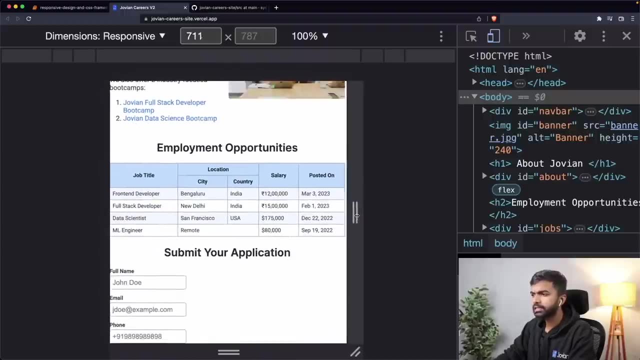 This is a good way for you to inspect how things are going. You can see that definitely there's a big problem here. The table doesn't look good at all on mobile and it starts to look a little better when we go into tablet or maybe even desktop screen. 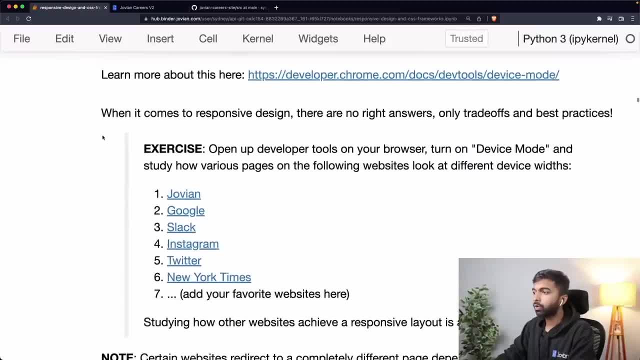 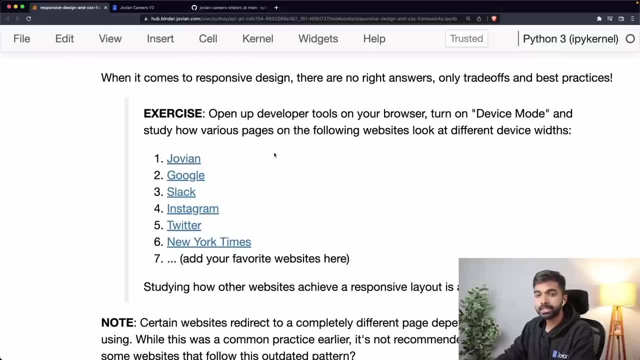 Okay, And one good idea for you would be to open up developer tools on your browser. turn on device mode. Let's see how various pages and websites look with different device widths. You can check out Jovian, So let's check out joviancom, our home page. 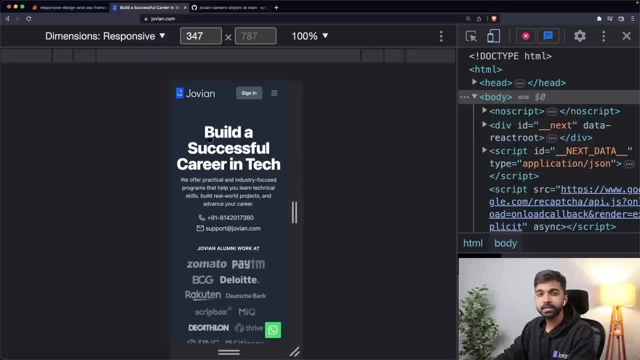 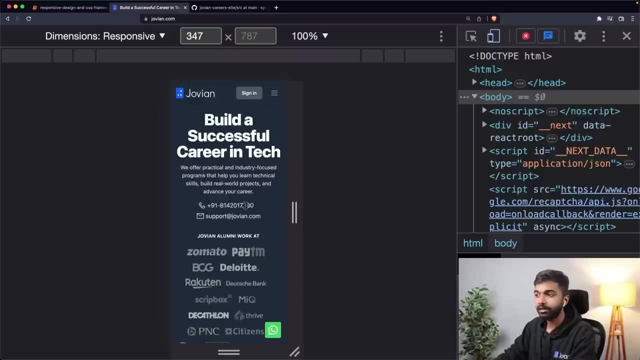 Let's start with mobile. This is what it looks like on mobile. So, on mobile, we just have this text, We have this explanation here. We have these two things and you can see that the text is centered on mobile. Then we have this logo cloud and then we have a form below it. 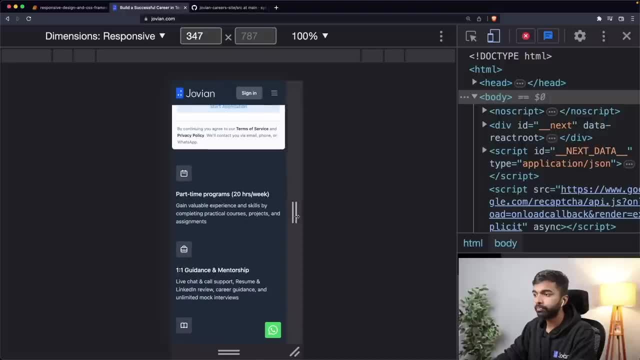 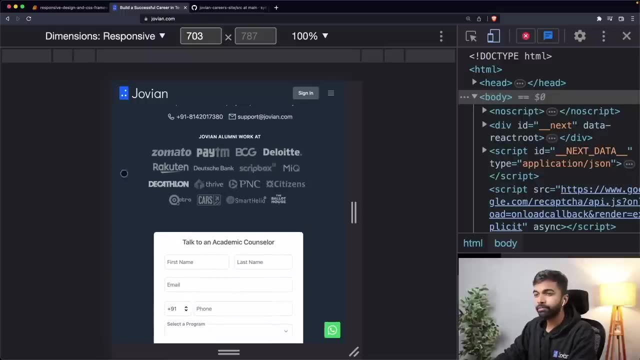 And then we have all of these benefits that are shown, Okay, Okay, Shown one below the other As we go. on a tablet screen you can see now that the text is still centered and but now we've put a maximum width for the logo cloud. 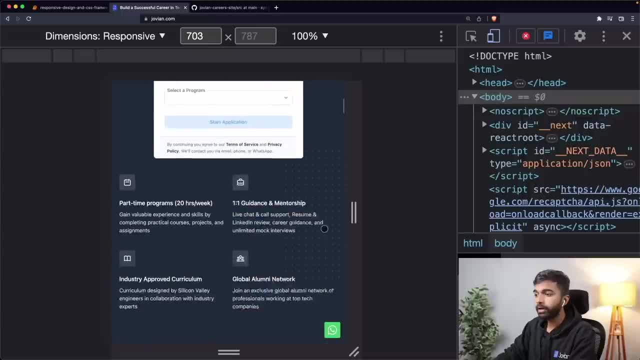 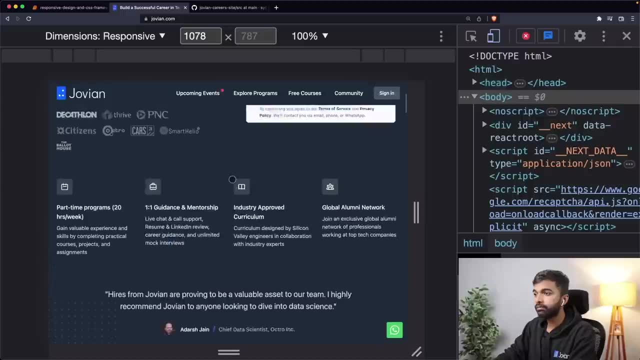 We've put a maximum width, We've added space around the form and now we are showing two of the benefits on the same row. As we go further, let's go into a desktop screen. So now we've gone beyond the 900 pixels or so, which is a desktop screen or a large screen. 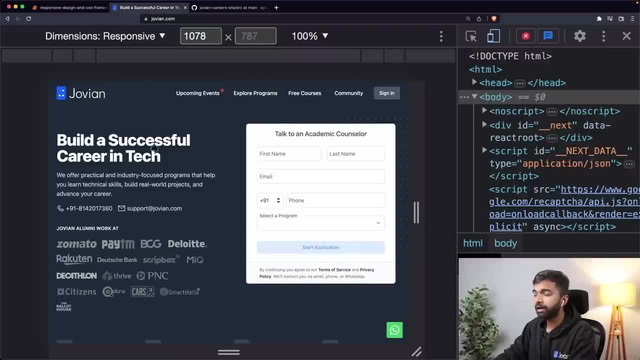 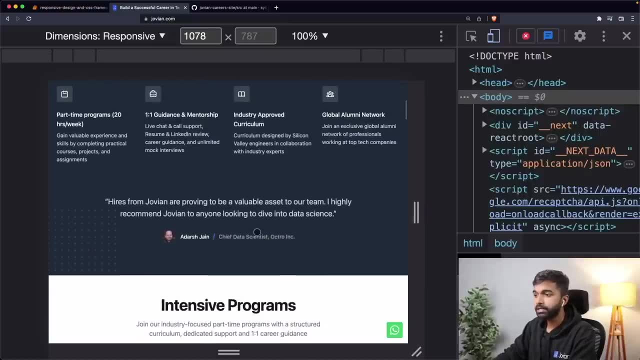 And now you can see here that we have a bunch of options here in the nav bar. Then we have left text and we have a form here, And then we have now all four benefits listed on the same page, on the same row, And of course there are similar changes that are there on each section as well. 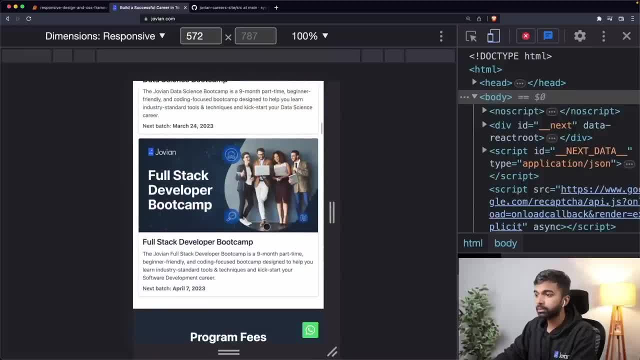 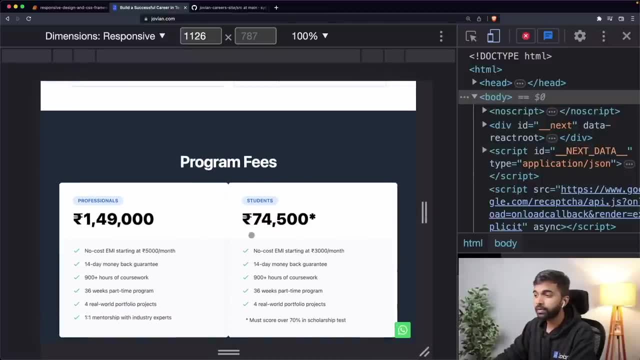 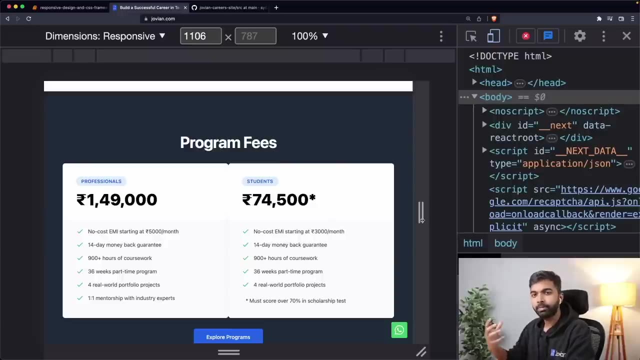 You can see here intensive programs. here goes one in each row instead of two per row. Okay, You can see that. okay, maybe this is something we need to fix. So it looks like in the pricing dev we haven't taken care of spacing and this is what happens when you are. 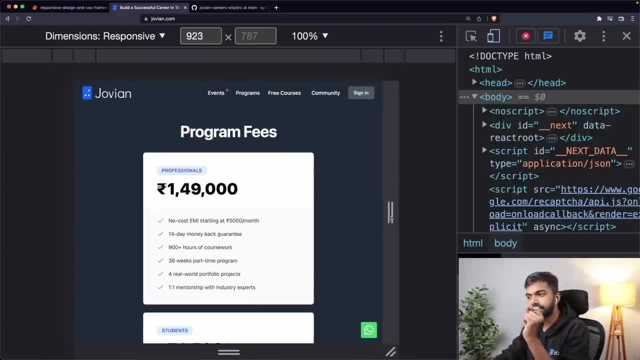 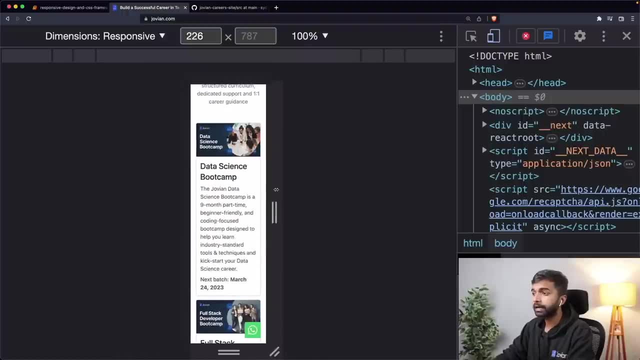 building Responsive websites. There will be slight cases here in there, a certain place, where you've not thought about how things should look, and you will have to go and fix it, And that is why it's important to check across the entire range of bits. 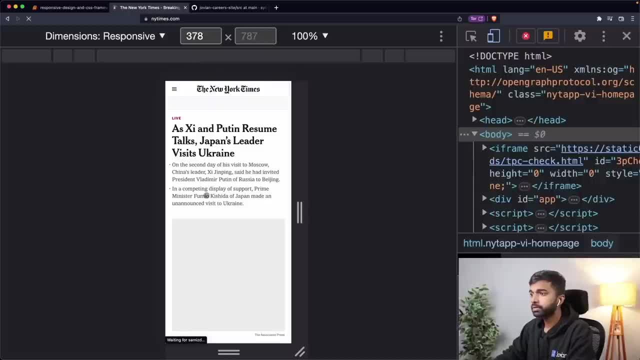 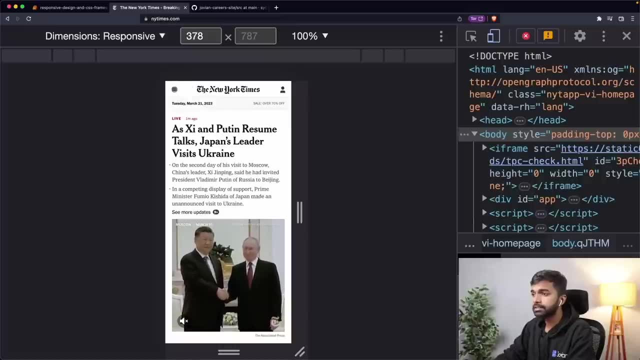 Okay, Let's check another one: NY timescom. So this is what the New York times looks like on mobile. You have a very little space on mobile. That's why there's just this title And then there is this nav bar. 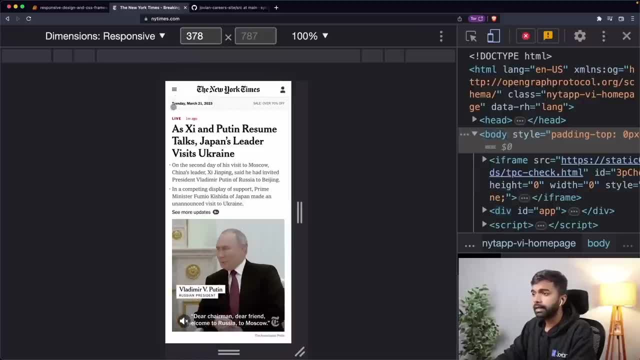 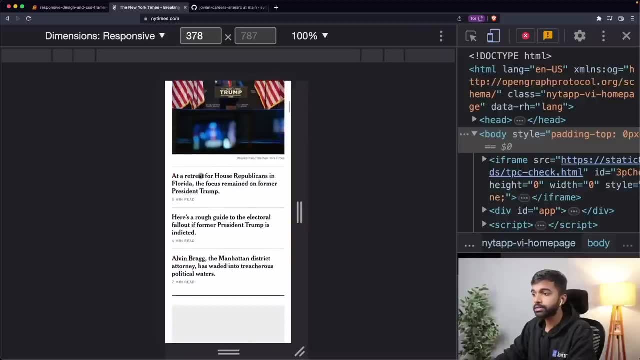 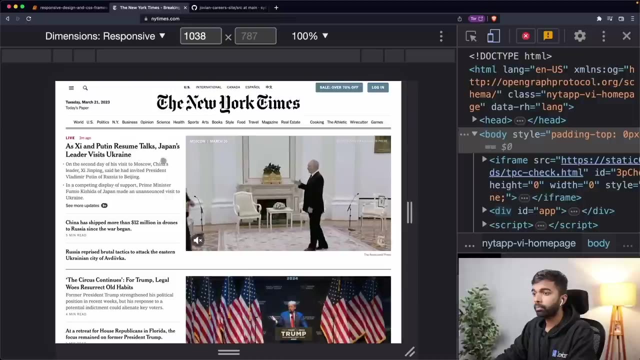 We'll touch on how to show these nav bars at a later point. And then there is just this date and there's the sale offer going on, And then there is this one story and then another story below it, and so on. But as you start to increase the width, you can see that now we go from one story to multiple stories. 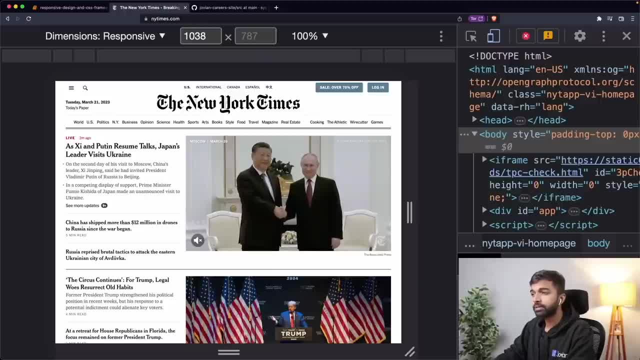 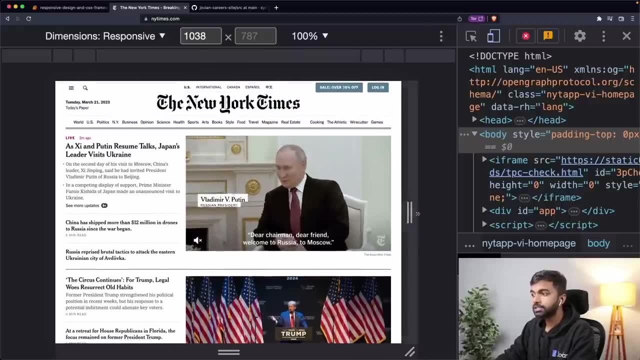 And we also get this second bar here which opens up a bunch of categories, And we also get something here on top. We also get, maybe, a login button and all. So things change significantly based on the screen that we're on Right. 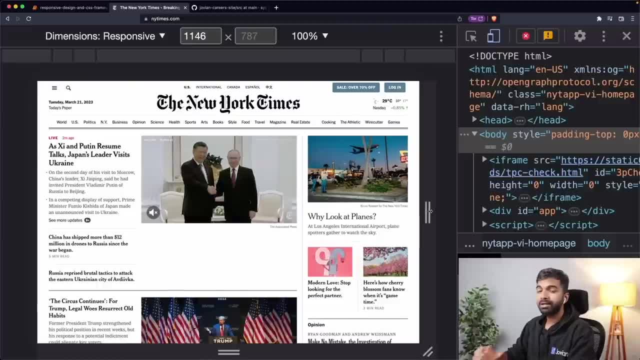 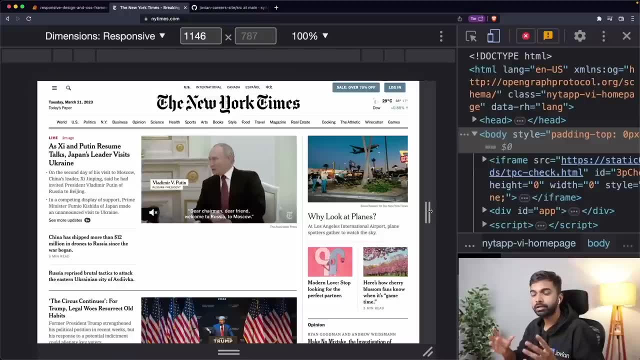 And you can see now we go into three column layout when three columns are available. So a lot of times Is spent by designers deciding where exactly to change the layout, what the breakpoint should be and what the structure should be for the site. 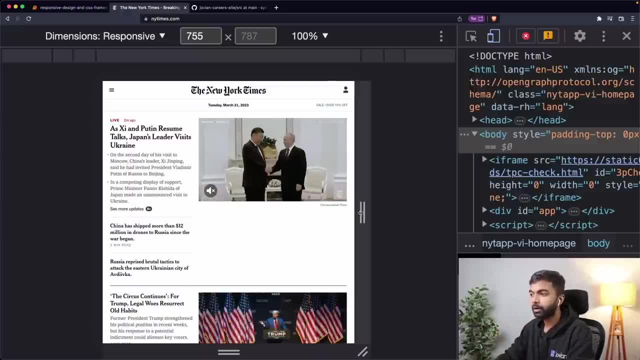 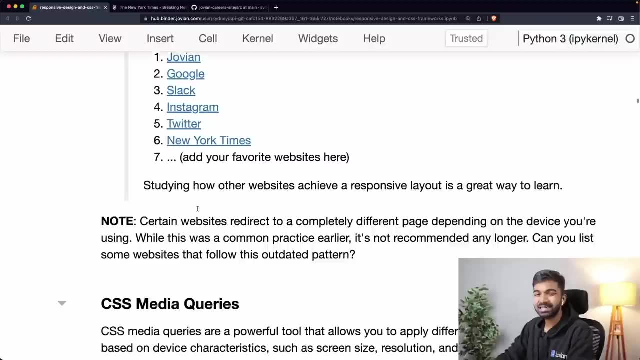 And really this is where a lot of the time is spent Just fine, tuning small things and testing things carefully, Okay, But I encourage you to maybe explore a few more sites and see how they work. Now, certain websites redirect to a completely different page when you try to access them on mobile. 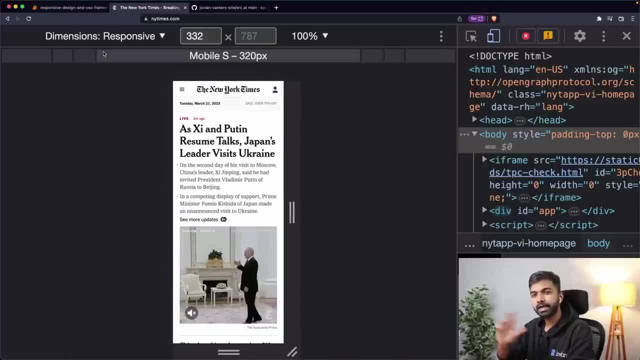 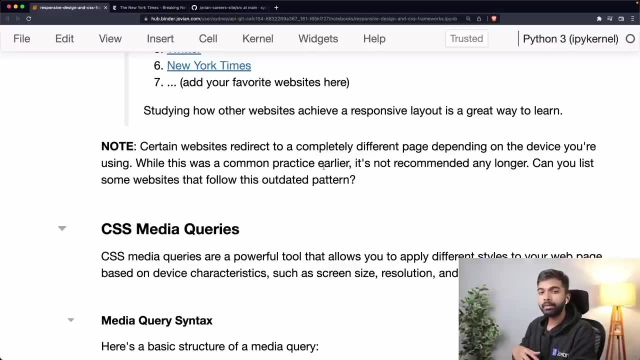 For example, if you were to open Gmail on mobile, it will redirect to a slightly Different page or show a completely different design. That was a common practice earlier, but now that there are many tools to, or many techniques to, build completely responsive layouts, 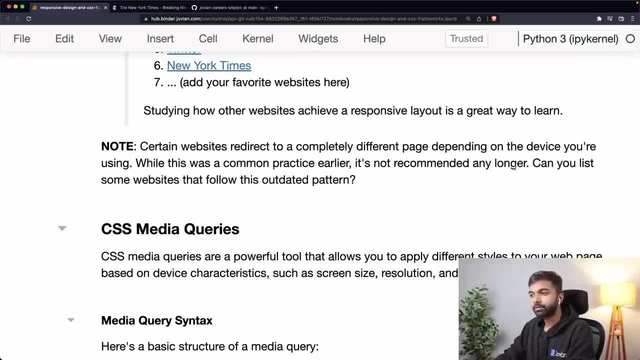 It's not recommended any longer. Try to find some websites which follow this outdated pattern and avoid it When you are building websites. instead, what you should do is build something called a mo, take something called a mobile first approach, which is what we look at today. 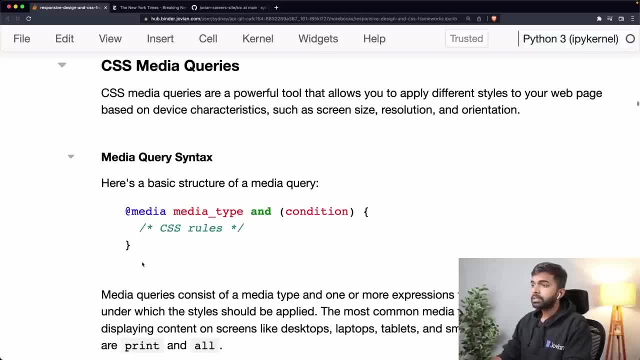 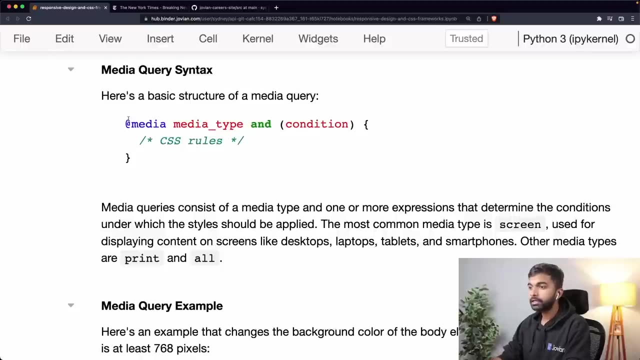 Let's talk about CSS media queries. This is: media queries Are a powerful tool that allow you to apply different styles to your webpage based on device characteristics such as screen size, resolution and orientation. And here is the basic structure of a media query. 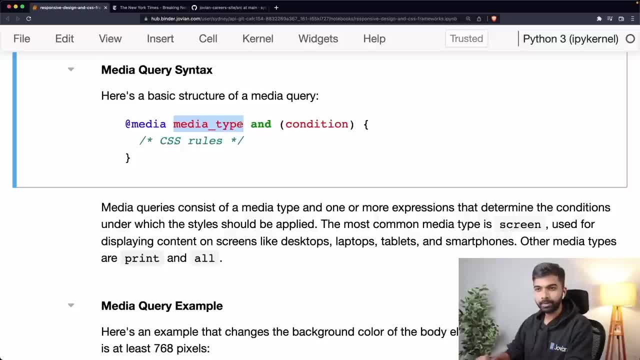 You say at media, and then you specify a media type, and then you specify a condition and you can have one or more conditions, And then you open up these brackets and inside these brackets the CSS rules that you write will only apply when you are looking at the 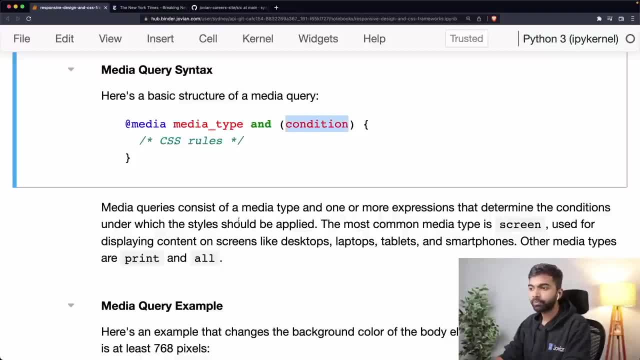 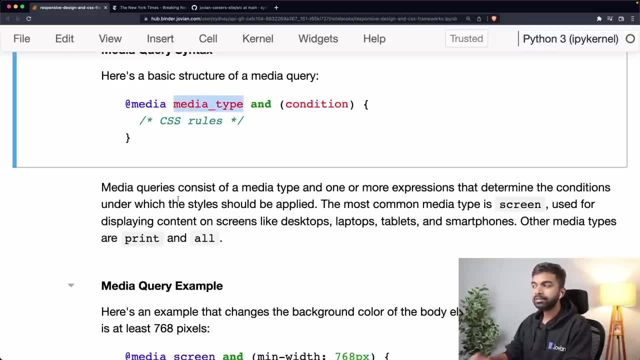 This particular media type and you're looking at this particular condition Now, when you're working with responsive web design, the media type is almost always going to be screen. So there are three types of media. There is the screen, and then there is print, and there is all. now print is used. 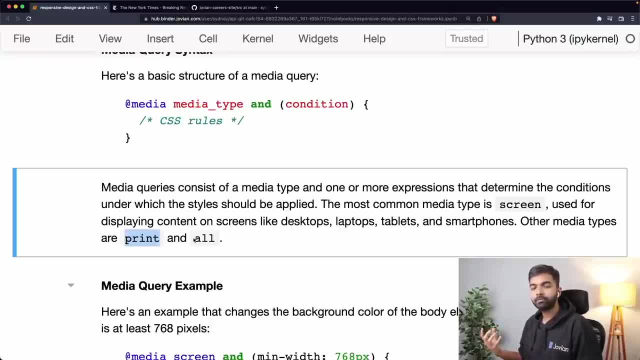 The print media type is used when you try to print a page or export it as PDF, which is not something we're going to look at today. So in our case, the media type is almost always going to be screen, or it can even be all. 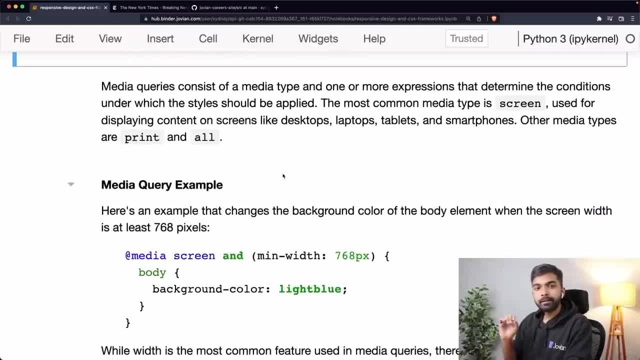 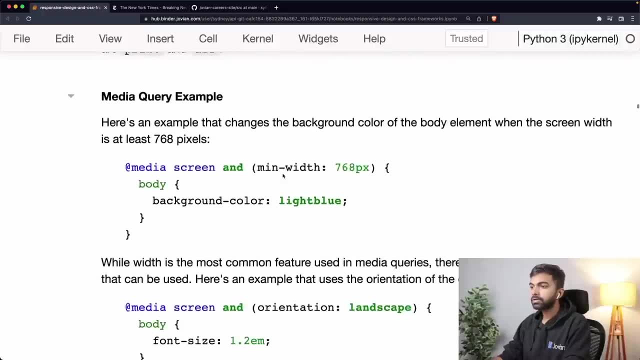 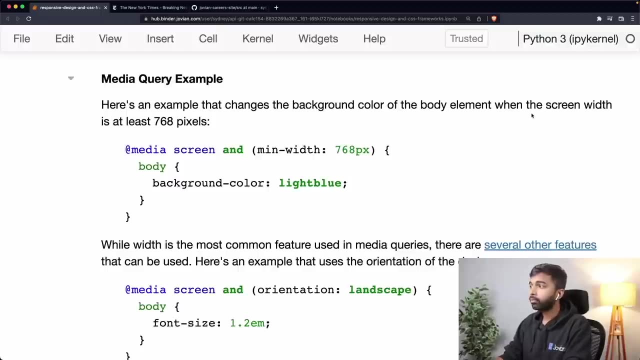 And the condition is something that you can set based on the width of the screen or the orientation of the screen, or there are a bunch of other properties that you can use. So here is an example. Let's say we want to change the background of the body when the screen width is at least 768 pixels. let's say, on mobile screens we want to have a separate background. 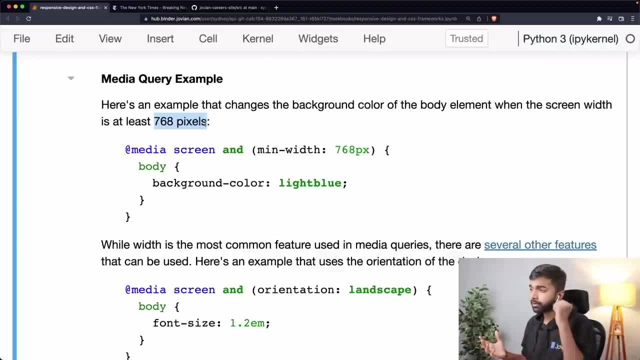 And then on on large screens or desktop screens, we want to have a separate background. So here is how we might do it: We can say at media, and then we can say screen, because we only want to affect the screen layout, not the print layout. 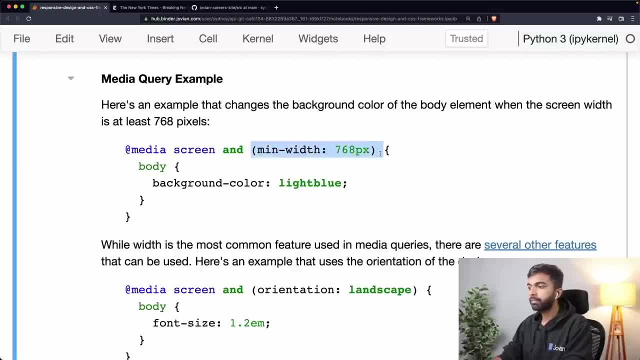 And then we can say, and, and now we can specify a condition: min width is 768 pixels. So when the minimum width of the browser is 768 pixels, then we can specify that the body should have a background color of light blue. 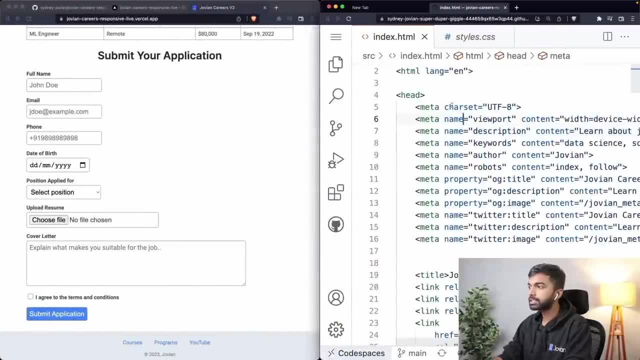 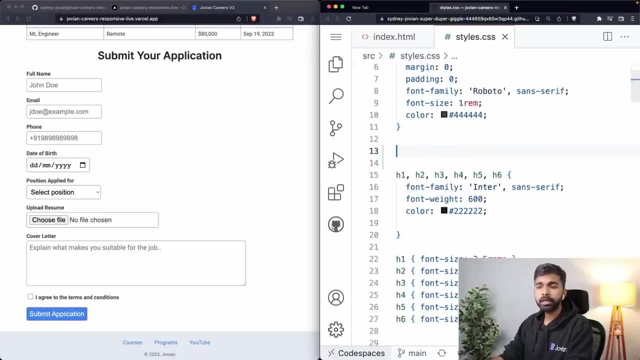 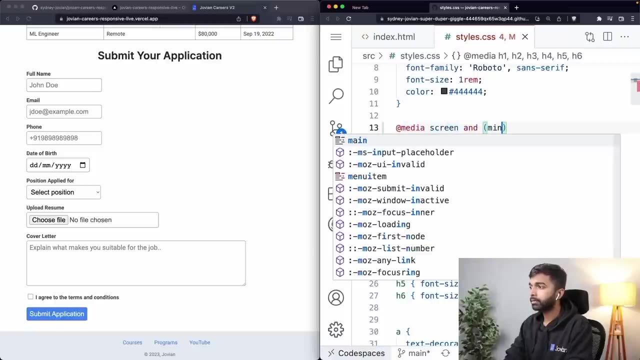 Okay, So let me just copy that and let me put that into my CSS file. here I am in my CSS file And right, maybe right below here, the main body declaration. I'm going to add this at media screen and min width: 768 pixels: 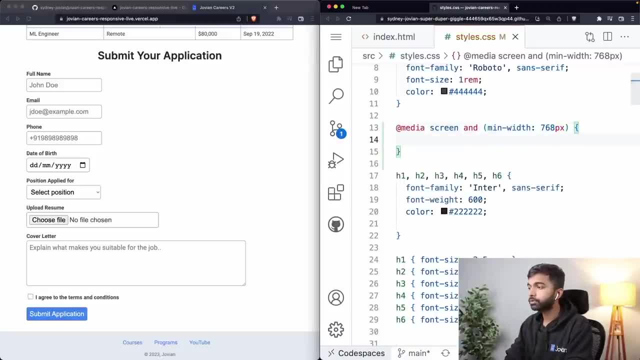 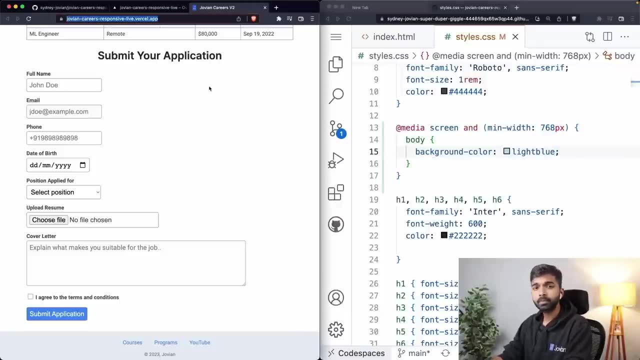 That means at a minimum width of 768 pixels. when the condition holds true for the body, I want the background color to be light blue. Okay, Right now I need a way to actually preview the changes that I just made. What I'm looking at here on the left is the deployed website, but I'm making changes in my GitHub code space. 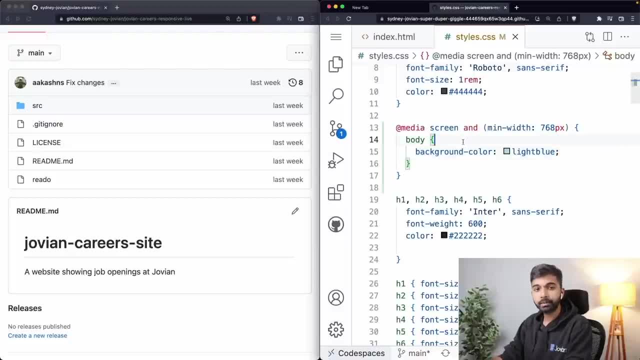 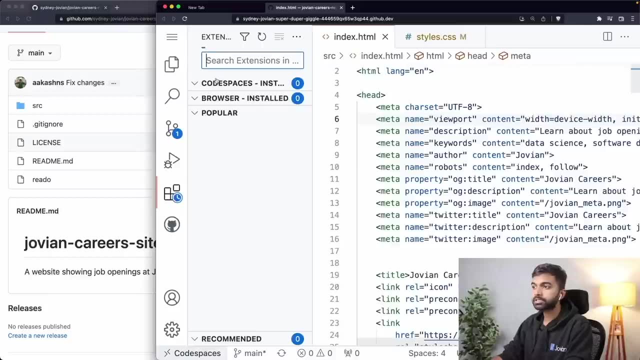 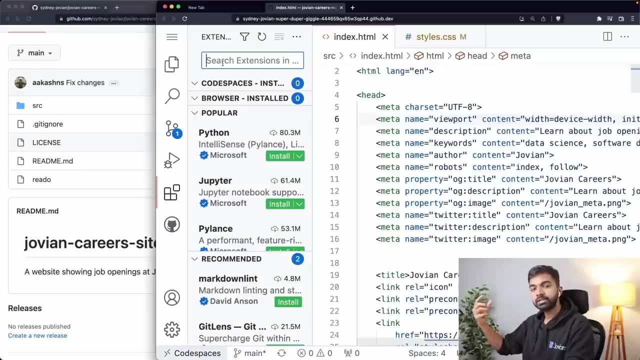 So what I need to do is I need to launch this GitHub code space, this indexhtml file, in a preview And remember, for preview we actually use an extension called live preview because our code space is a system somewhere on the cloud and we need to now view the HTML code. 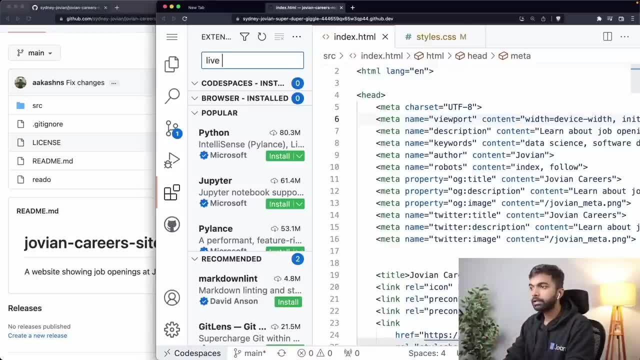 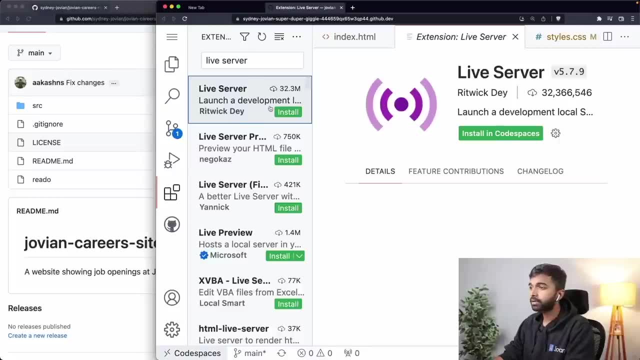 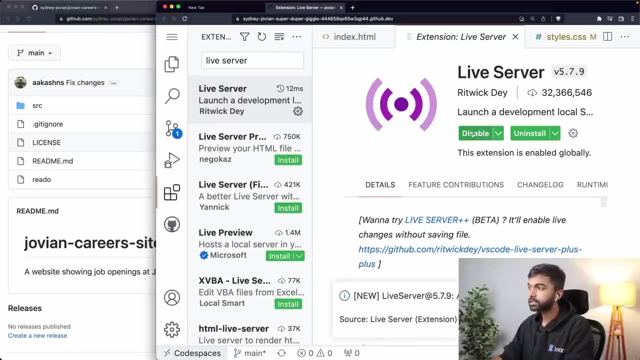 In our browser As a web page, and for that we can use this live server extension. Okay, So let us open up the live server extension. So search for live server by Ritvik day and click install and code spaces. And again, all of this is covered in the previous tutorial. 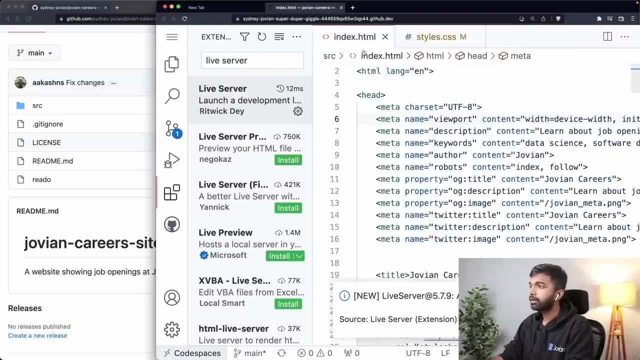 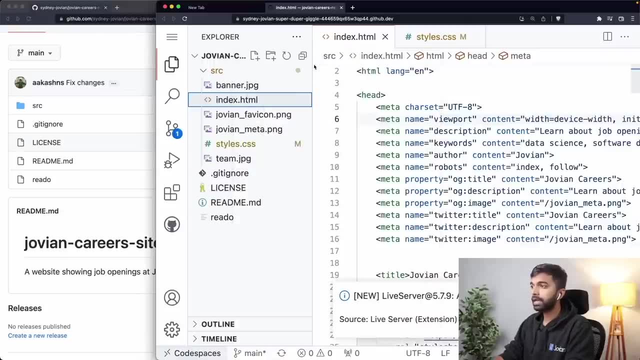 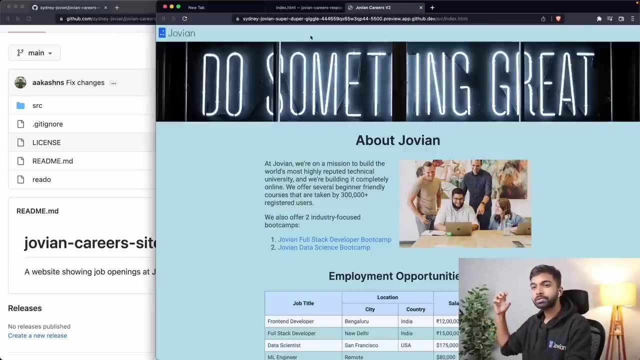 So you should review that in case this doesn't make sense. And now let's come back into indexhtml and let us right click on indexhtml and click open with live server. Okay, So now what this is doing is this is going to set up a simple server which is going to serve the file for us so that we can now view it in our browser. 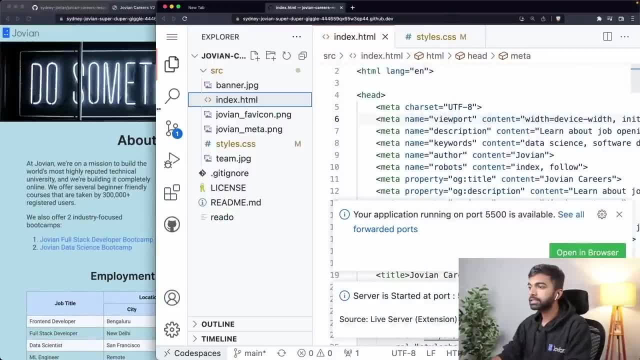 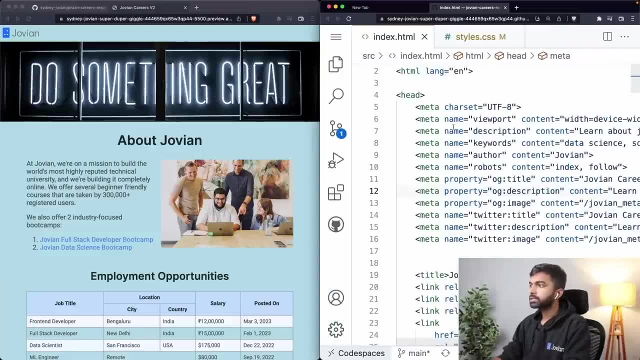 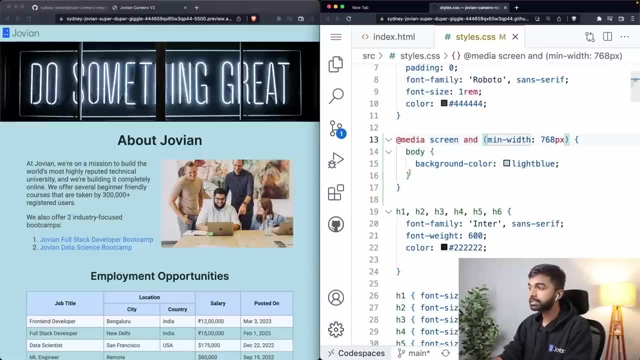 And let me just bring that and put that here on the left. Let's bring this back here on the right. Okay, Now I have this stylescss and I've mentioned here that whenever the screen width is more than 768 pixels, my body should get a light blue background. 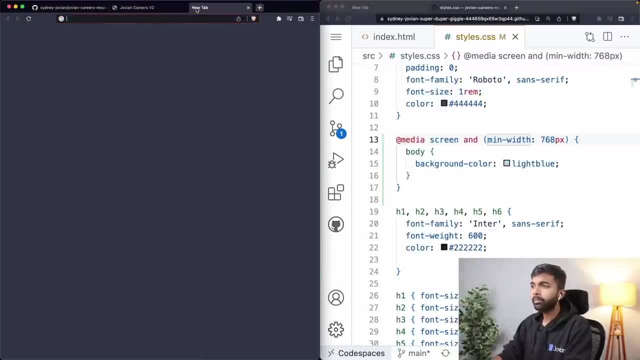 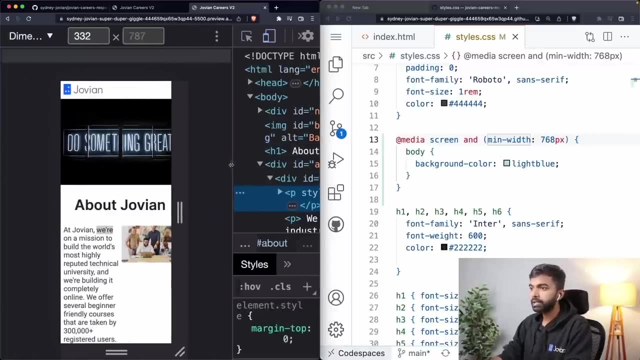 Clearly it has gotten a light blue background, which is fine. Okay, It's not looking good, but it demonstrates what we're looking for. but let me go in here and let me also click inspect And let me just reduce the width of the screen. 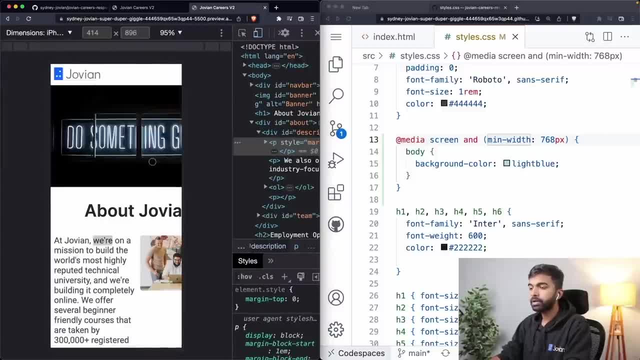 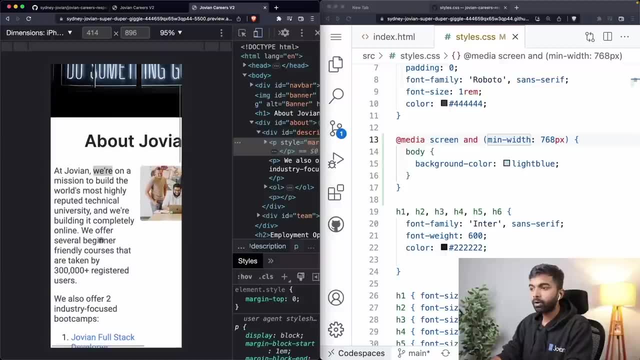 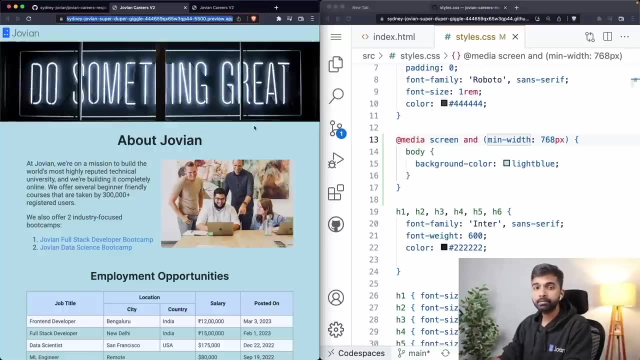 Let me reduce it down to maybe an iPhone 10 R. You can see that when I'm viewing the same page on a mobile device. on the mobile device it is still has a white background, but on this device over here it has a blue background. 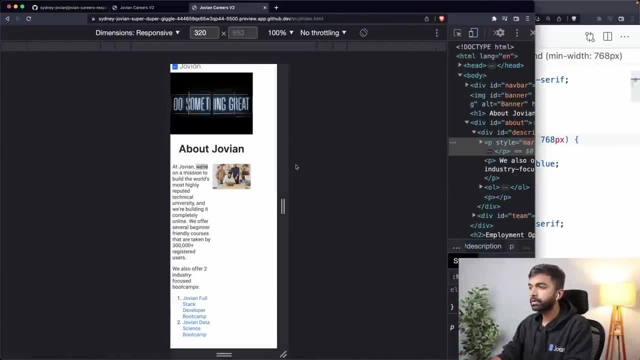 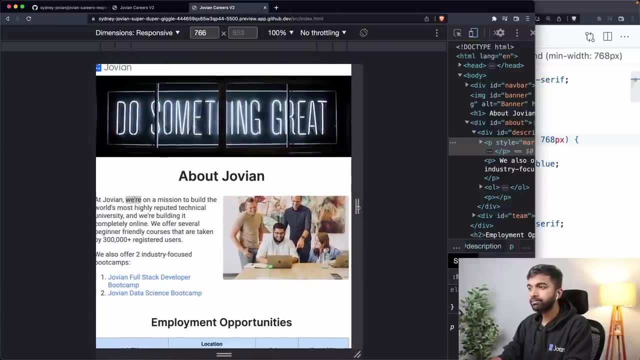 You can see the exact Change happens at 768 pixels. So as I increase, you can see that just before 768 pixels it is still white, but at 768 pixels it turns blue. So you can do all sorts of things like that. 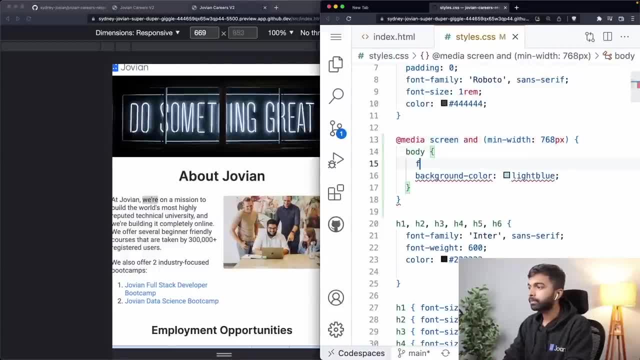 Let me change another thing. Let me maybe set the body font size to 10 pixels or to 20 pixels. Let's just make it 24 pixels, so that the font size also changes drastically. So here you can see that I have below 768 pixels. 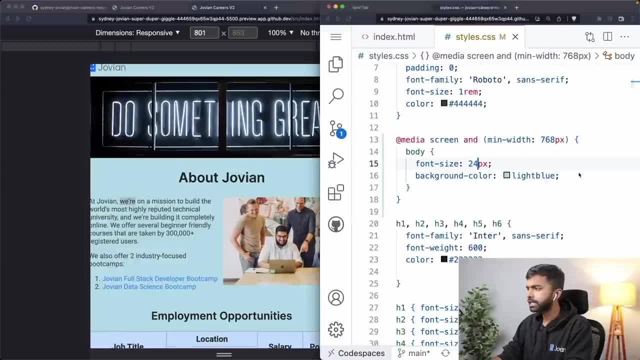 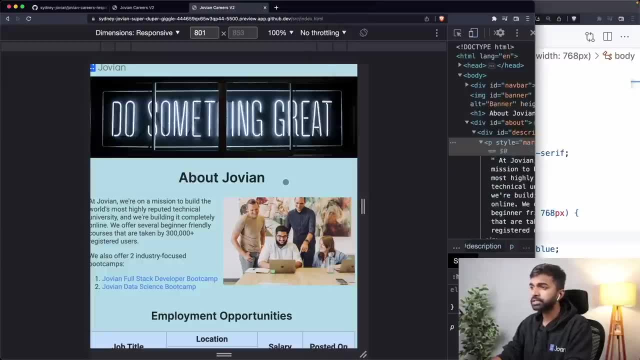 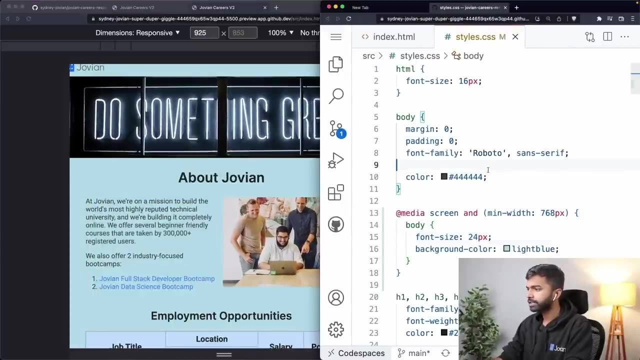 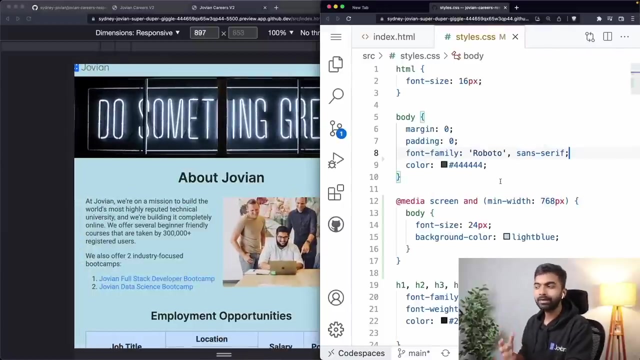 And then, as soon as I cross 768 pixels, the body font size should change. Well, okay, Didn't I just need to reload the page? Maybe? yeah, maybe, if I just remove this it might change, but it doesn't seem to be changing right now. but it will, uh, depending. maybe I just have to like set the uh. 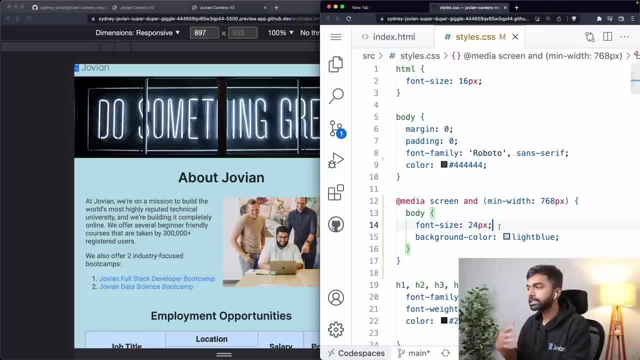 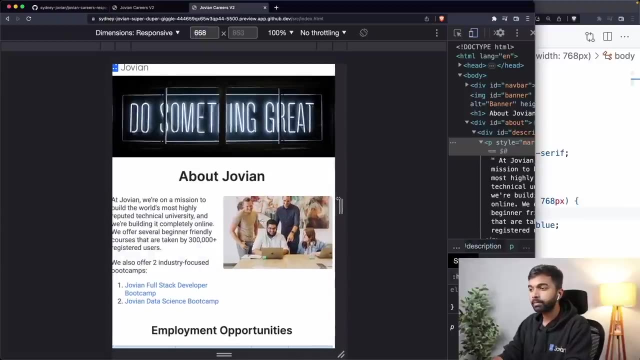 properties properly, but you can set any property here and the font size can change significantly for that particular tag and or for that particular selector based on what property you set here. Okay, So for now I'm just going to revert it. and: below 768 pixels, the background is white. above 768 pixels: 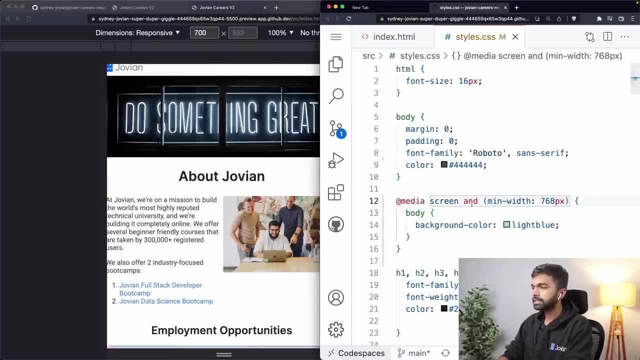 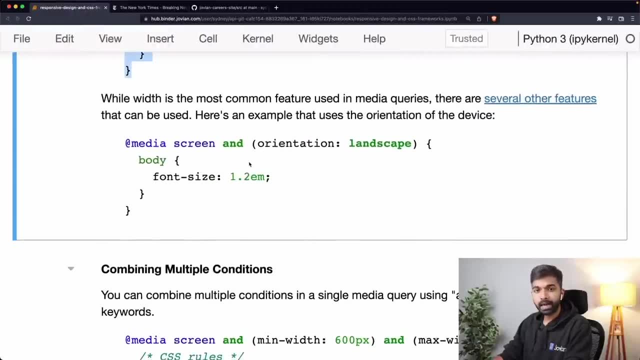 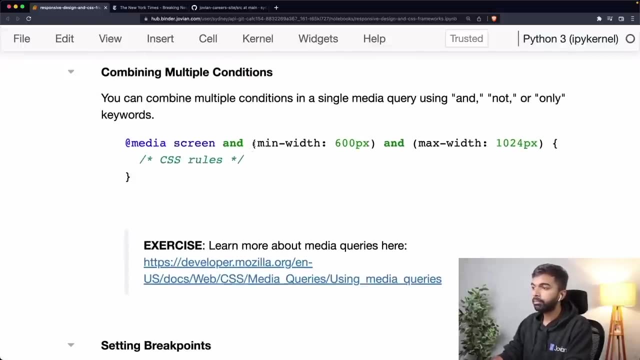 The background is blue. So that is how you use media queries, And let me just get rid of this for now. but one other thing you can do is also Combine. Combine a bunch of conditions So you can say something like this: that you want a particular CSS rule to apply only between min width of 600 pixels and max width of one zero to four pixels. 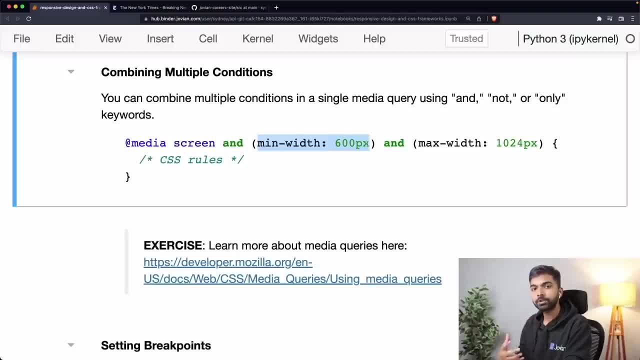 So at 600 pixels you want it to start, And that same set of rules you want them to end at one zero to four pixels. You can imagine how, using this, you can set up maybe one layout for under 400 pixels, one for 400 to 600, one for 600 to 800, and so on. 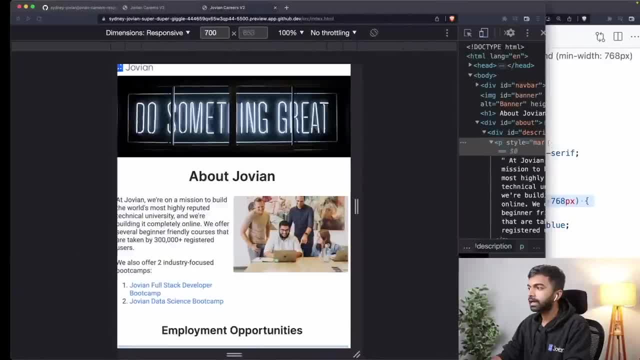 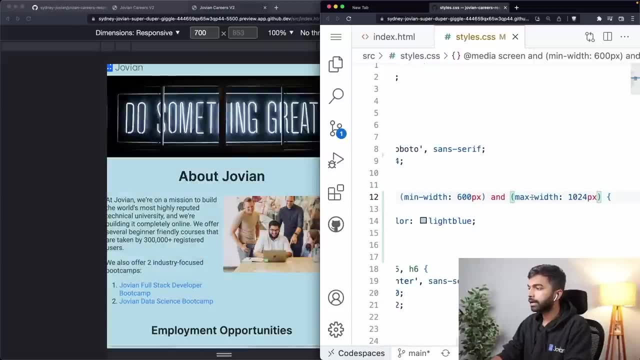 Right, Let's look at an example of this. Let me just take this and let me put it in here. Now I'm going to put a couple of layouts. I'm going to say that at: let me just make it 400 and 800, 600 pixels, just so that we can actually view the changes very easily. 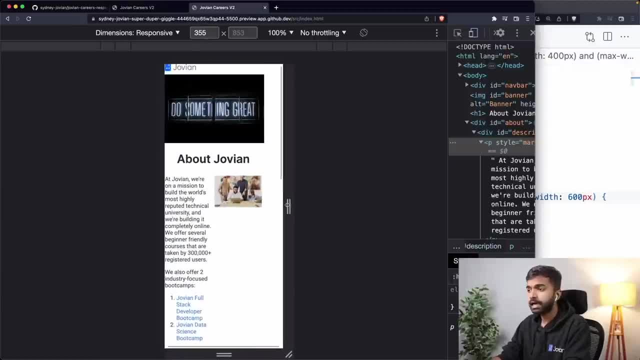 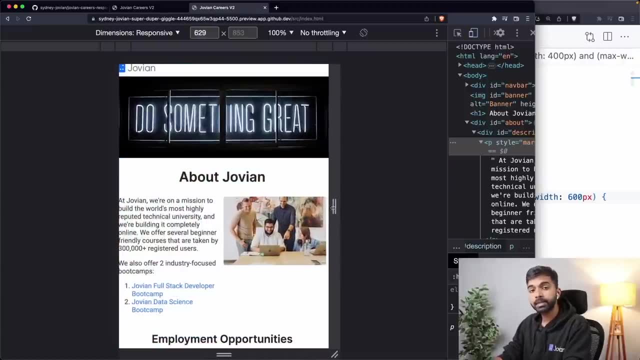 Now what I'm saying is that under 400 pixels I have a white background And then as soon as I touch 400 pixels, the background turns blue. But as soon as I cross 600 pixels, the background does white again. 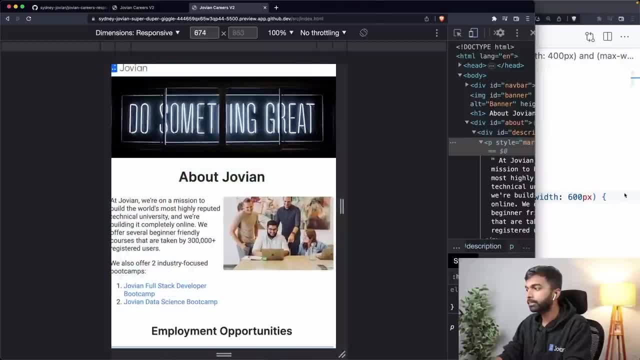 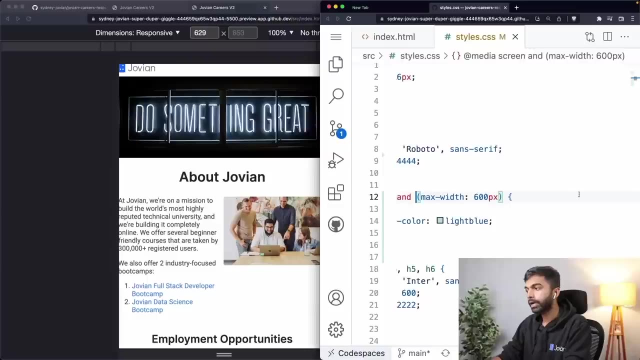 Okay, Do you see what's happening? You can combine multiple conditions Like this, and you can also do something like this. Let's say I want to only have a condition for max width. So then I want to say that only under 600 pixels the color is blue, and over 600 pixels the color is going to be white. 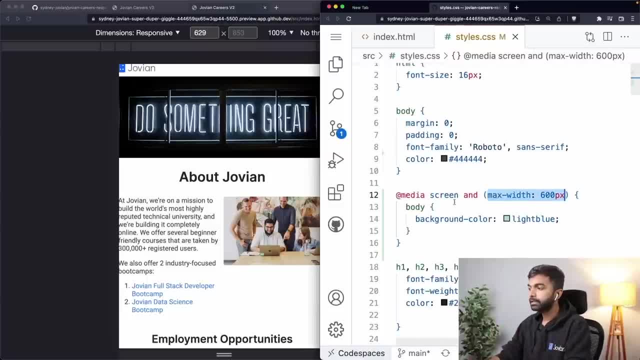 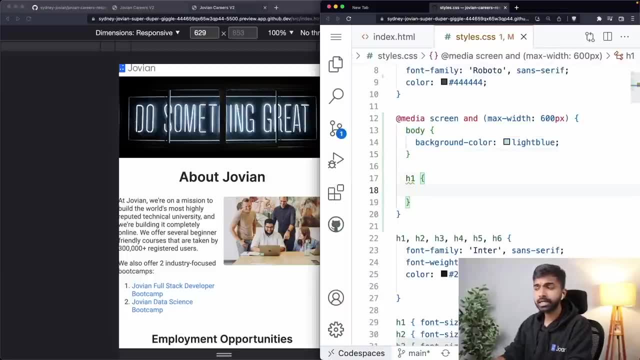 So as long as this condition or all conditions are satisfied, these CSS rules apply and I don't just have to put body here. I can maybe put change the edge. one color is the edge, one size here again put maybe change some other size here as well. 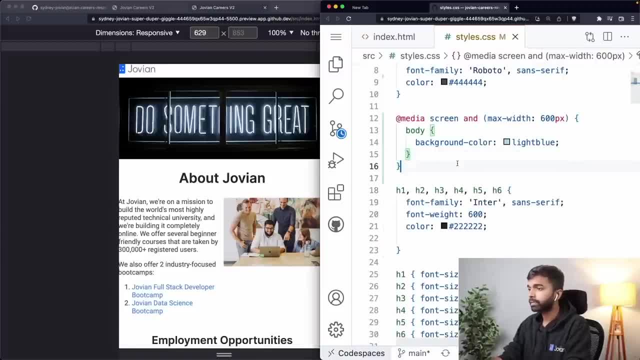 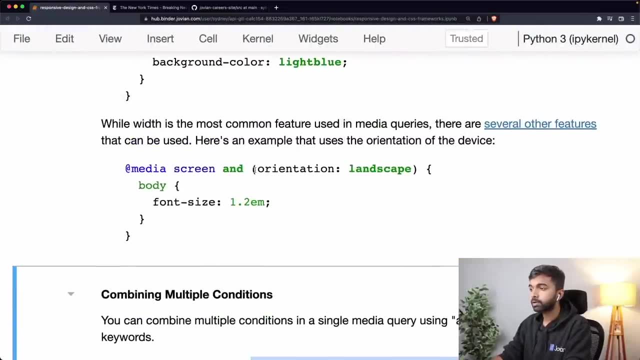 So I have all those controls That I can modify. Okay, Now of course you don't only have to look at the screen size, You can also use the orientation. So let's say, you want to use a certain font size only in a certain orientation. 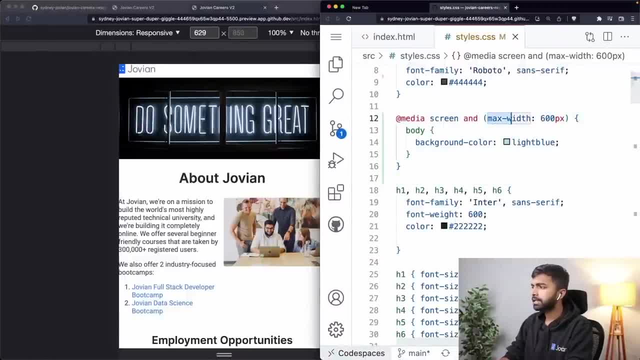 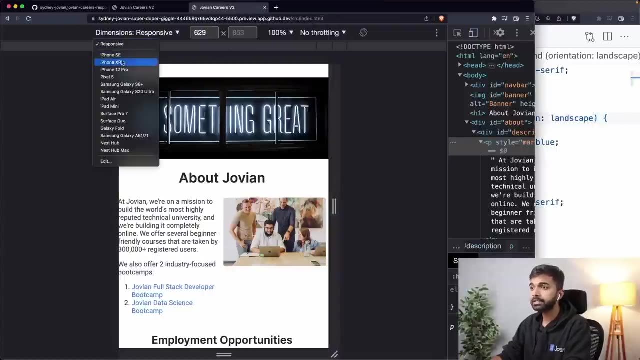 You can do that too. Let's maybe try that. So only in the landscape orientation, we want the light blue color. So orientation, landscape and the orientation is also. orientation Is also Okay. So let's go to iPhone 10 R and let us change the orientation here. 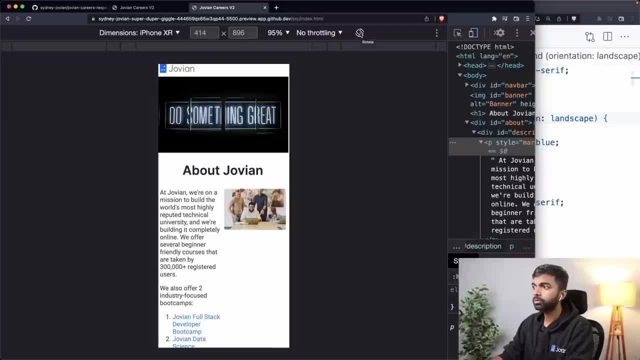 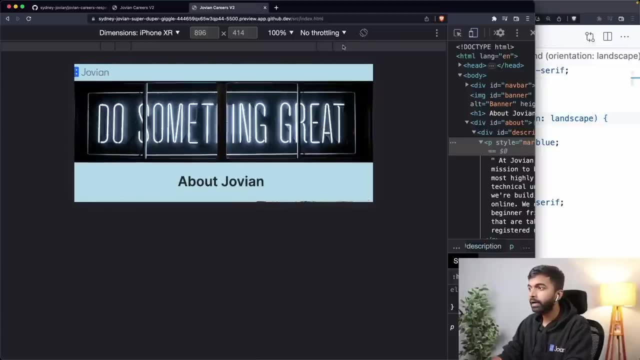 So there's a button here. You can see that. there's a button right here to change the orientation. You can see that now this is in landscape orientation and in the landscape orientation it has a blue background and I can change it back to the portrait orientation or the vertical orientation. 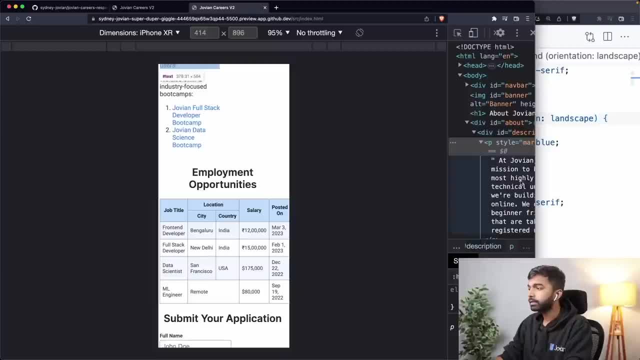 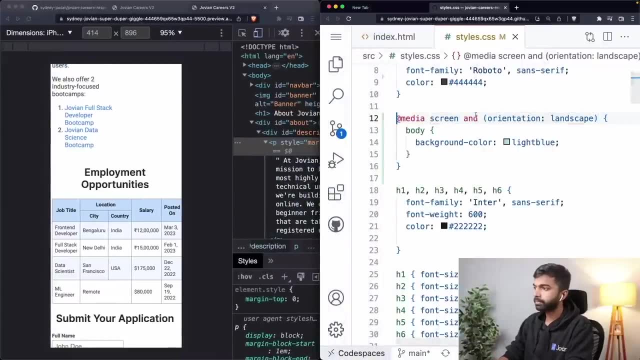 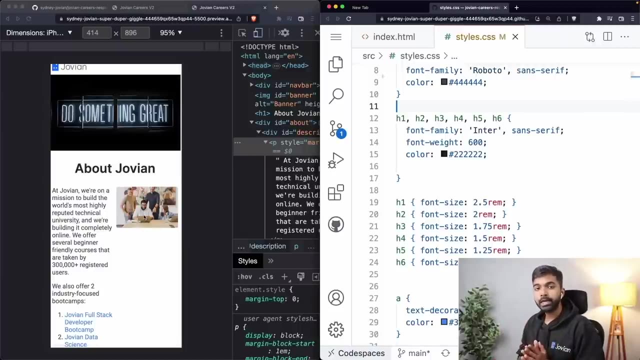 And in this case it does not have the blue background Right. So let's bring that back And let us get rid of this. So that is how media queries allow you to change the layout of a page at various breakpoints, And that is what we're going to use today. 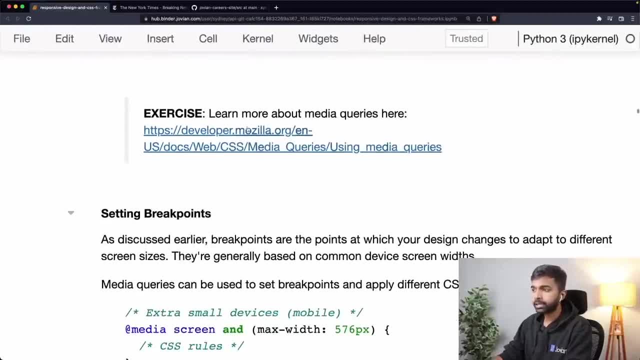 Okay, You can combine multiple conditions and you can check out some information about media queries here, but we've covered the most common use case. You'll be using the screen media type and you will be using maybe the max width or min width to set breakpoints. 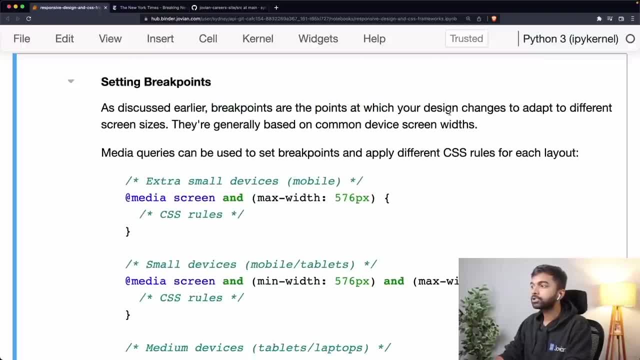 Specifically, as we said earlier, breakpoints are the points at which Your design changes to adapt different screen sizes based on the designs that your UI designer has given you. you may have to set some breakpoints, and these are generally set on some common device screen widths. 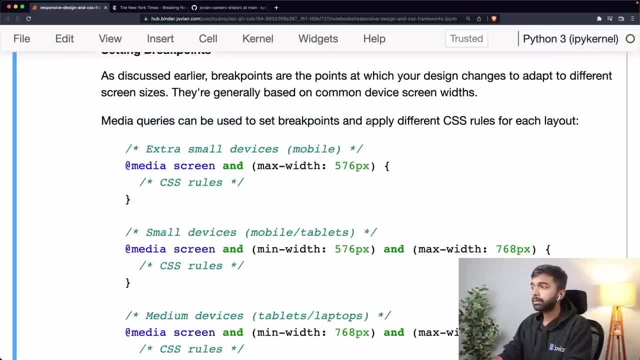 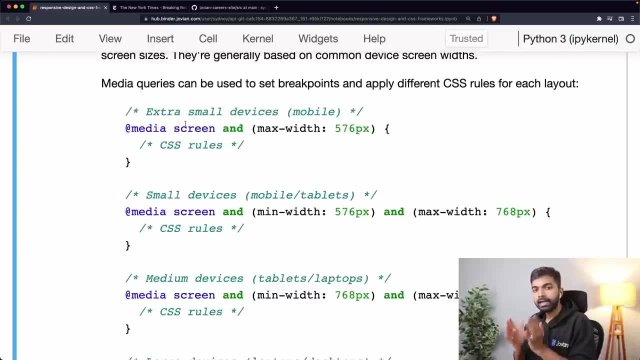 So media queries can be used to set breakpoints and apply CSS rules for each layout. For example, if you want to write completely separate CSS for mobile, tablet, laptop, desktop and large desktop screens, you may do something like this. You may have one section. 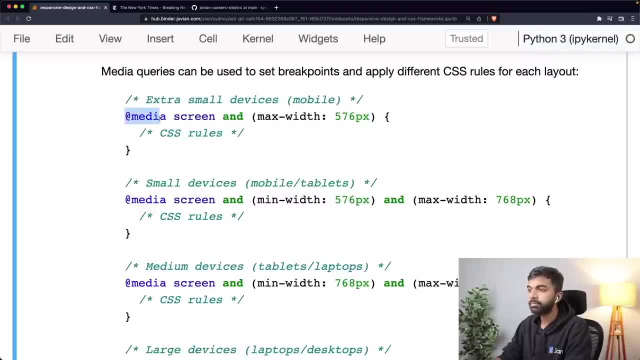 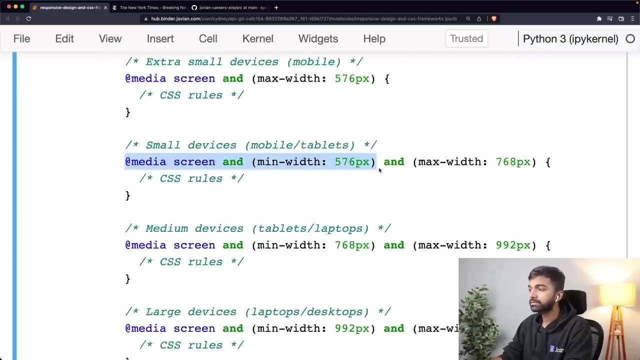 In your CSS file, which only deals with mobile screens. So you may say media screen and max width 576.. So under 576 screen width, all these rules are going to get applied. Okay, Then you may have maybe another media query here called media screen and min width as 576 pixels and max width as 768 pixels. 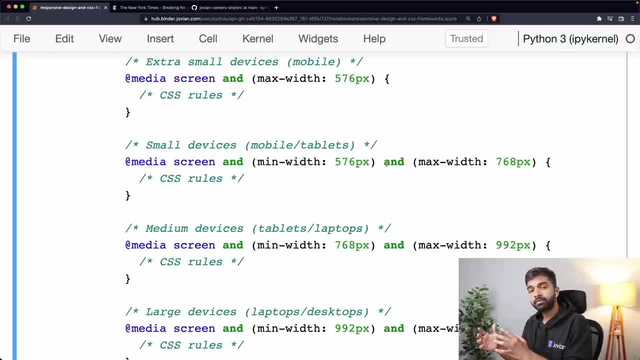 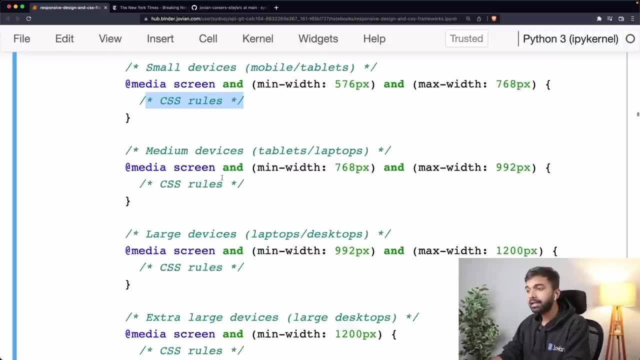 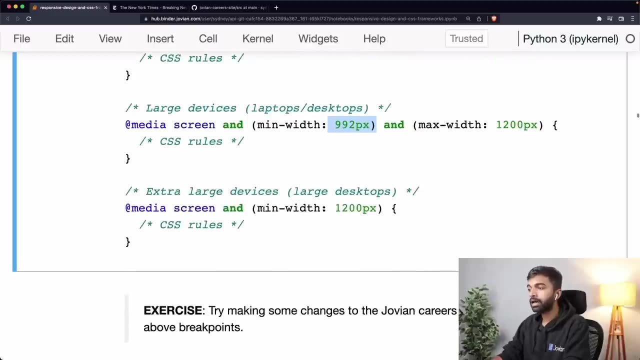 So between 576 pixels and at maximum width of 768 pixels. So between these two widths, All this, all these CSS rules will get applied, And then you may have maybe another one between 768 and 992, and you may have another one between 992 and 1200, and maybe you may have one for 1200 and higher. 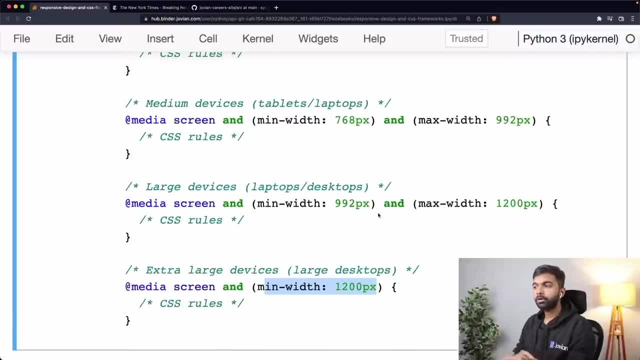 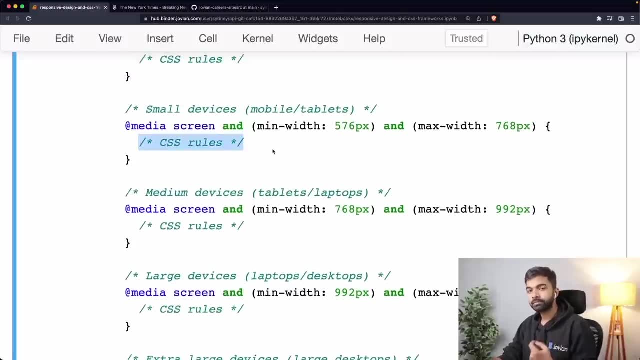 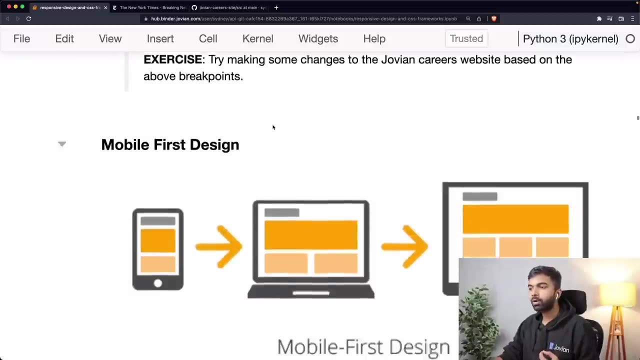 Right. So, depending on how many breakpoints you've decided on for your website, you can set up these min and max conditions, and then you can write completely separate rules for each of these. Okay, So this is one way you can go about doing things, but a slightly better way is what is called mobile. 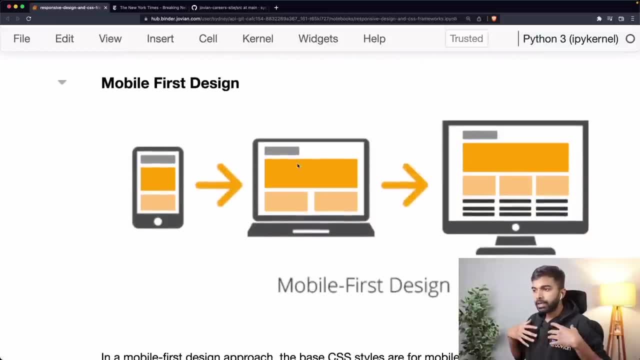 First Design. So the way you should be building most web pages today is by starting out with a mobile design. So first you should just design your web page, or build your web page for mobile and then slowly enhance that same web page to make it look good on, uh, on a tablet and on a desktop screen, and maybe on a large desktop screen as well. 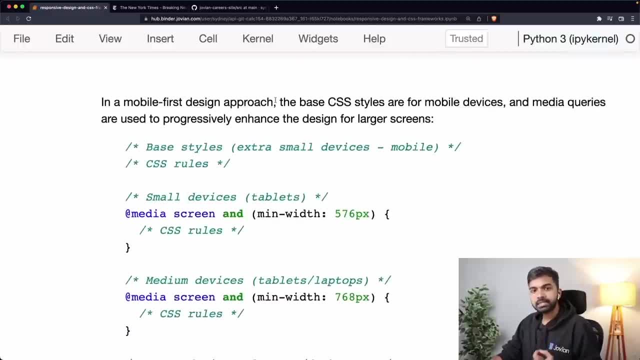 Right. So in a mobile first design the base CSS styles are for mobile devices, So you do not have What media query for the mobile devices. you just write all the base CSS styles and apply that to mobile devices And then media queries are used to progressively enhance the design for larger screens, right? 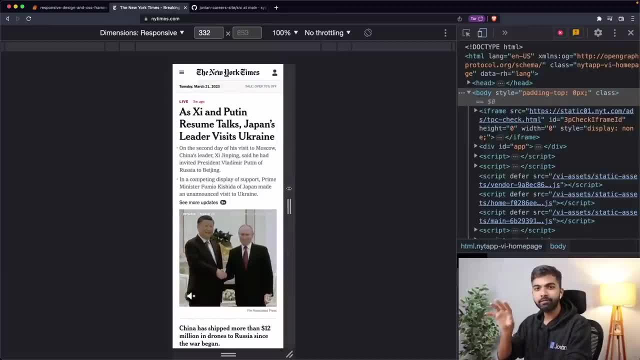 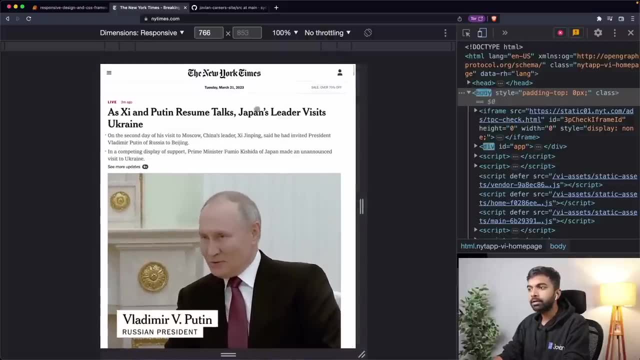 What you're basically trying to do is you're going to implement this design first and then, slowly, you are going to add a break point And then, at a certain break point, you're going to maybe make, you're going to maybe change this layout and maybe go shift to a two column layout. 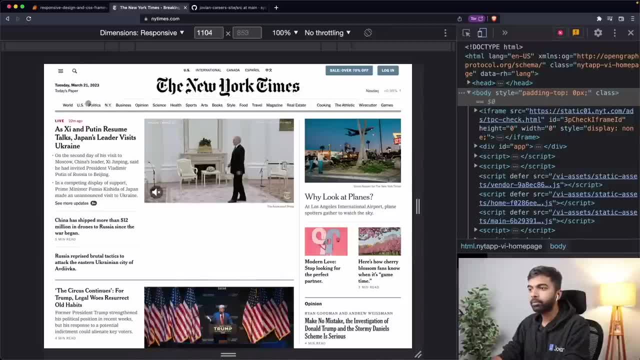 Then, slowly, you're going to add another break point And at that particular break point, you're going to add, Okay, A bunch of these categories, and you're going to shift to a three column layout and so on. Right, So that is what we're going to do. 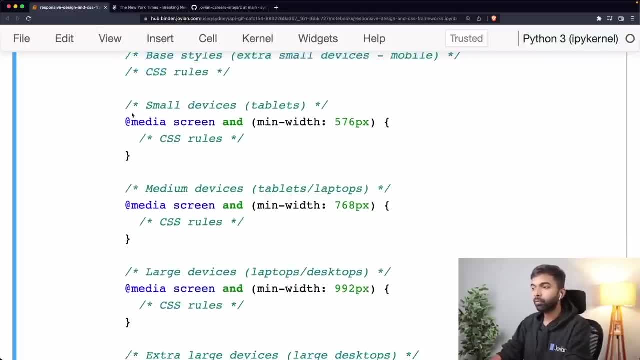 We are going to start with the base styles and then you can have whatever new styles you want to introduce. for tablets, You can simply say media screen and min width 576. So you're telling the browser: only for screens with more than 576 pixels apply these new CSS rules. 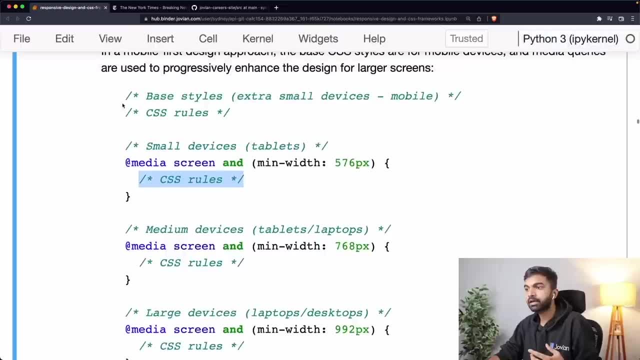 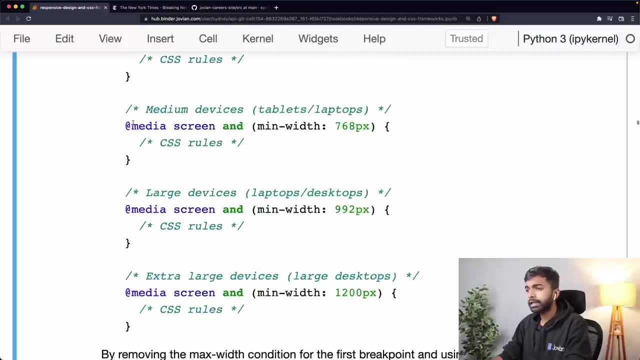 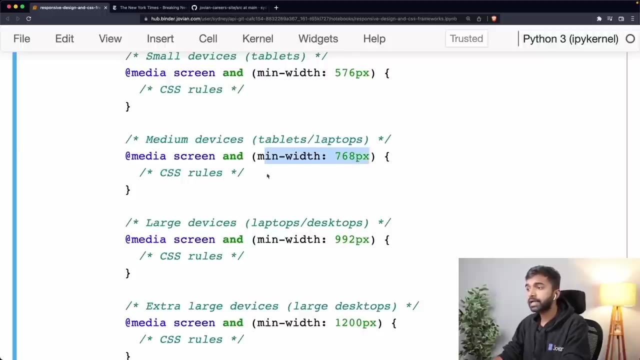 And some of these CSS rules will override the old CSS rules that have been set in the base styles. So that's how media queries are more selective, So they can override the existing styles. And then we have, similarly- these are a next set of a next set of rules- min width: 768.. 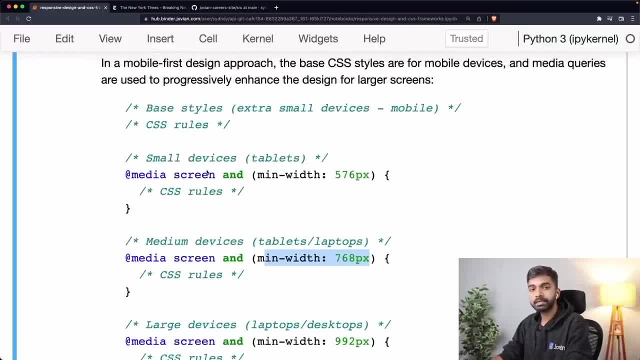 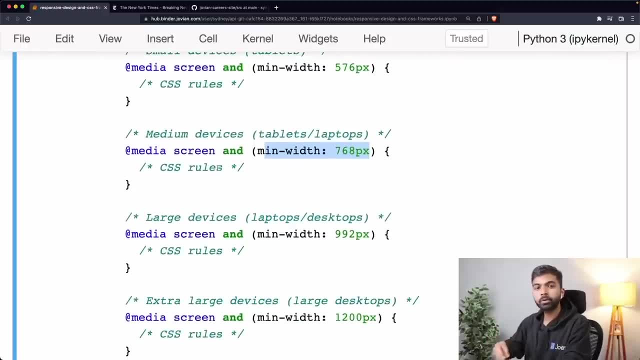 And these rules are going to override the rules that have been created in these and these. they also follow the order and they follow the specificity. That is how CSS works. So all these rules are going to override the previous rules that you have set. 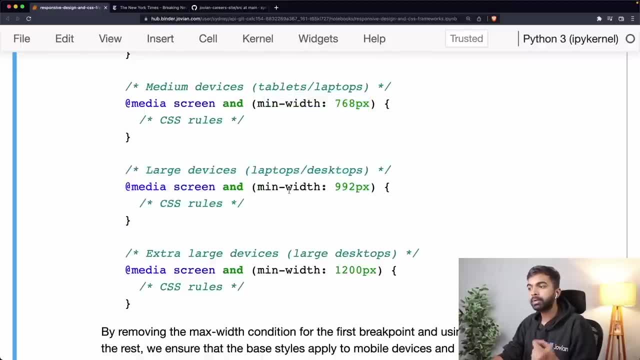 And then you can similarly have maybe another where you can say media screen and min width 992.. So only when the screen width Crosses 992, these new rules will get applied, only a selective set of rules, and they will override any rules that have been previously applied. 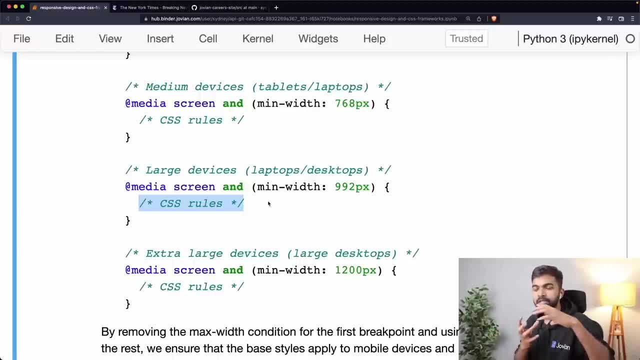 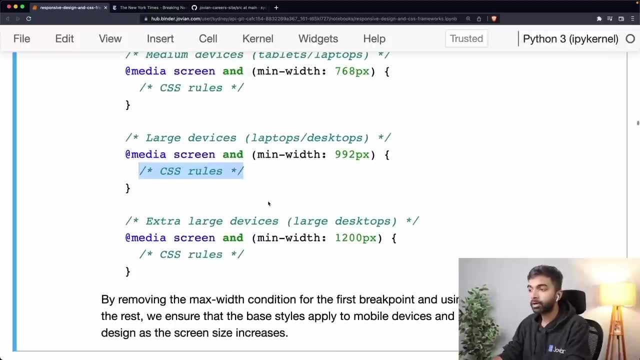 This way, you don't have to repeat a lot of CSS for every screen. Rather, you can start. you can start with the mobile design and you can just add a few properties here and there to make the website look nicer on tablet. And this is a great approach, because if you start out with the desktop layout and you try to compress it down to mobile, you're going to face a lot of difficulty. 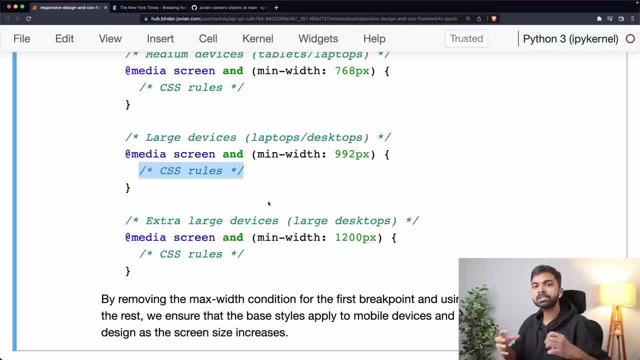 Rather, if you start out with the mobile layout, Often the tablet and desktop layout will simply either have more information or rearrange some of the things in a uh into multiple columns, And that is easier to achieve rather than taking more information and compressing it down into one call. 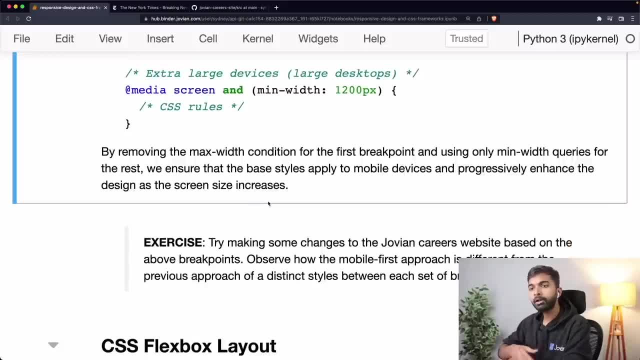 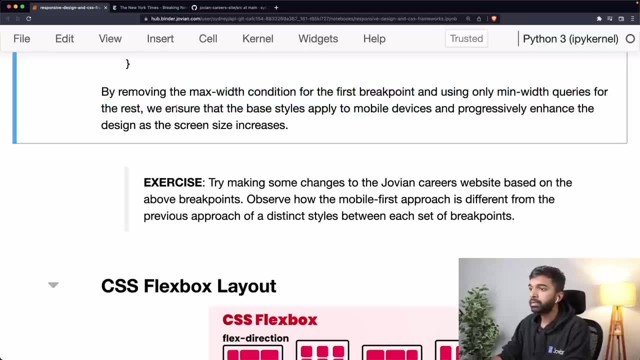 So, even as a designer, you should always start from the mobile layout and then slowly build out the desktop. So by removing the max with condition for the first break point and using only min with queries for the rest, we ensure that the base styles apply to mobile devices. 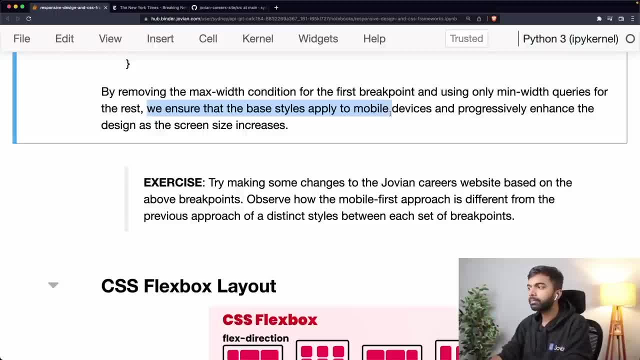 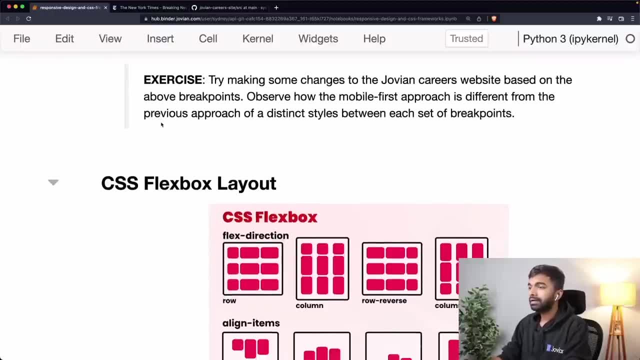 And then They apply to all devices further as well, but progressively we also enhance the design as the screen size increases. So Try experimenting with this. try setting up some of these breakpoints in the CSS file and experimenting with this to make changes to the careers German careers website, make it more responsive and observe how the mobile first approach is different from the previous approach, where you have different set of styles between each set of breakpoints. 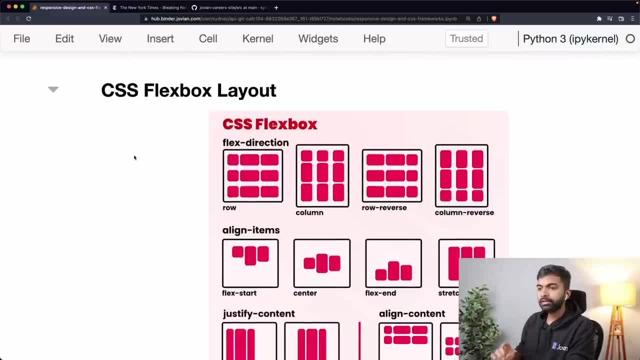 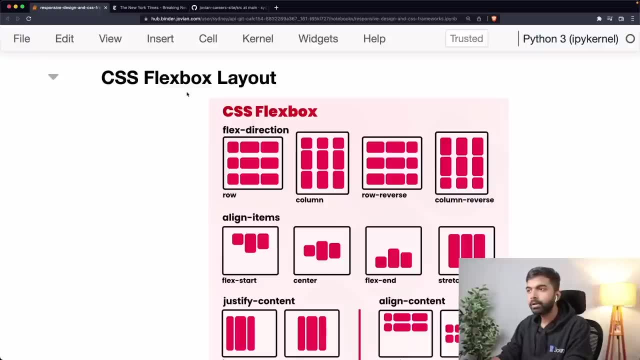 Okay, All right. So One other thing we need to cover before we go ahead and actually implement the mobile design is something called the CSS flex box layout, because it's not just that you're going to change the layout at certain breakpoints, between those breakpoints as well. 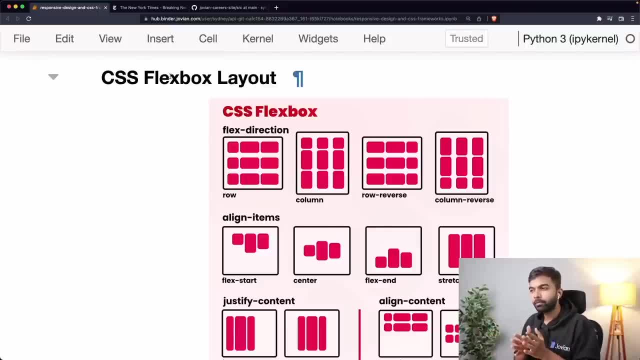 Sometimes you will have to make the layout a little more fluid, so that things go from maybe two columns to three columns or maybe the sizes of things increase and decrease and maybe you add space on the left and right. but to handle these kinds of fluid layouts 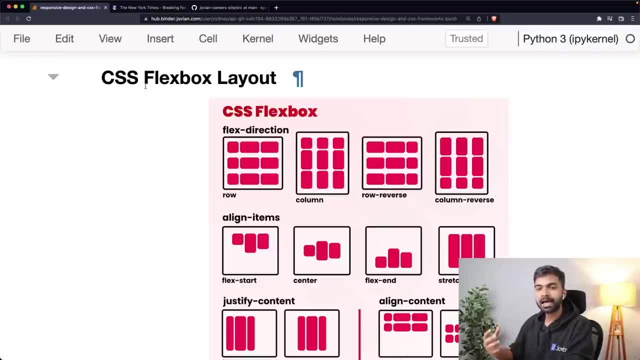 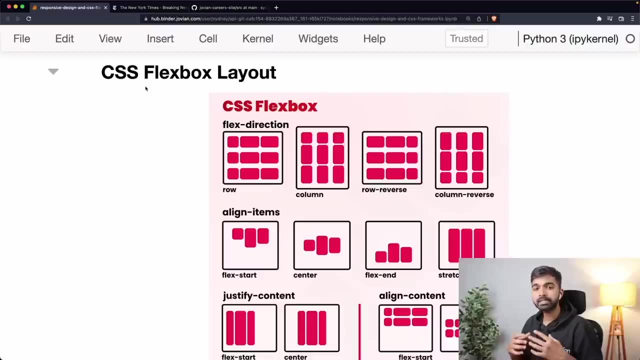 CSS has something called flex box, and this is something that was added to CSS about 15 years ago, about 14,, about 12 years ago, to be exact. So this, this is something that was added to CSS about 12 or 13 years ago when mobile layouts became more common, when mobile mobile phones became more common, to allow for creating fluid layouts that can be flexible and that can grow and that can automatically shift into multiple columns, et cetera, as required. 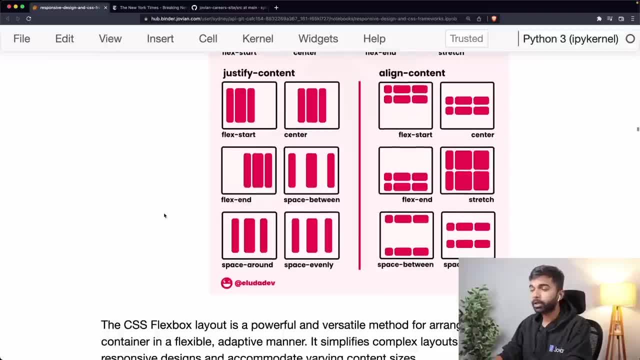 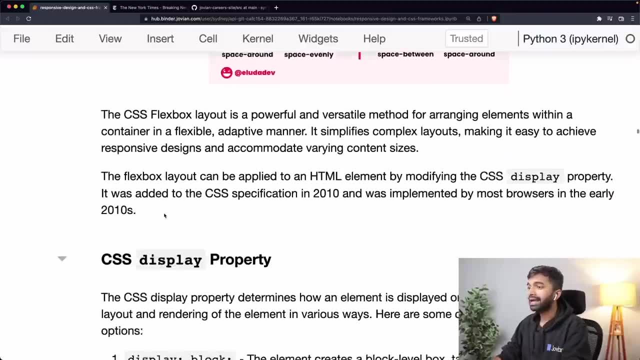 Okay, So we're going to look at the CSS flex box setup. We're going to learn a little bit about flex box. It's not a detailed flex box tutorial. We're going to learn the most common flex box properties and it is a versatile method for arranging elements within a container in a flexible and adaptive manner. 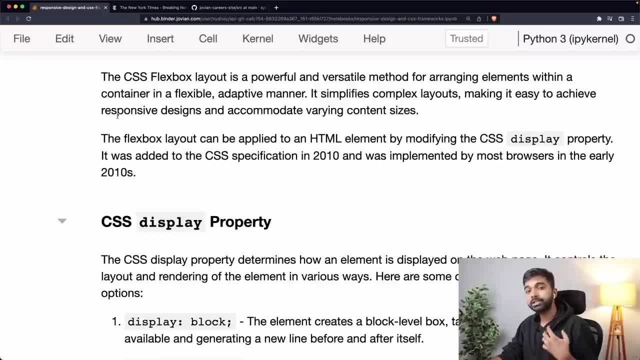 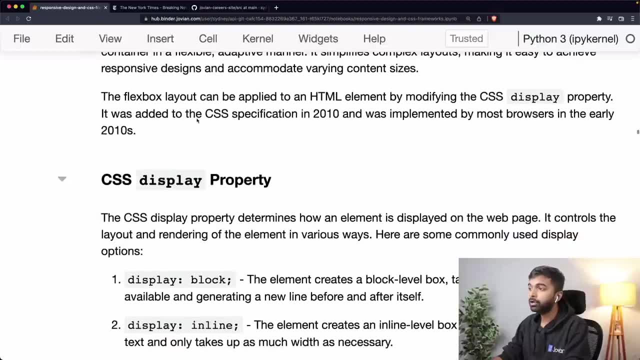 And it simplifies complex layouts, making it easy- making it easy to achieve responsive designs and accommodate of varying accommodate varying content sizes. Now the flex box layout can be applied to an HTML element by modifying the CSS display property And it was added to CSS in 2010, and it was implemented by most browsers in the early 2010s. and the CSS display property. 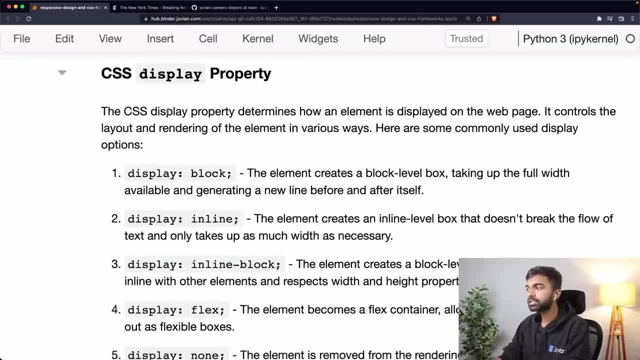 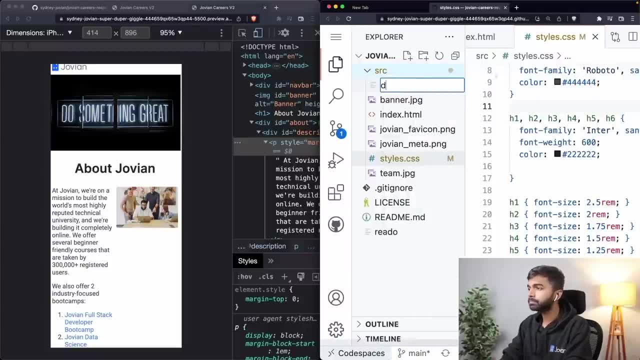 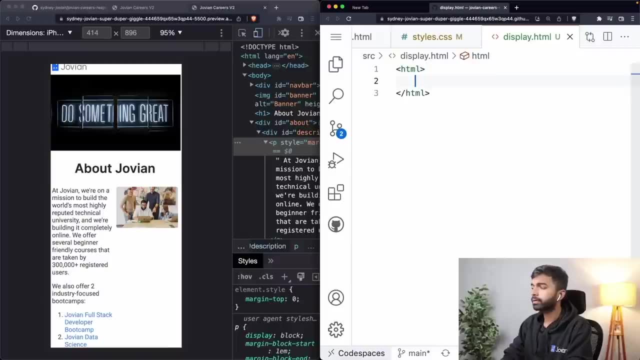 This is something that we've already seen here. It determines how an element is displayed on a webpage. So just to give you an example, I'm going to first just create a new file called display dot HTML, And in this file, display dot HTML, I'm going to create a bunch of, if some. let me just put in: 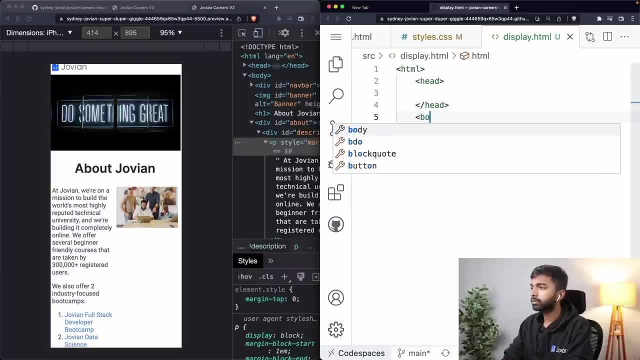 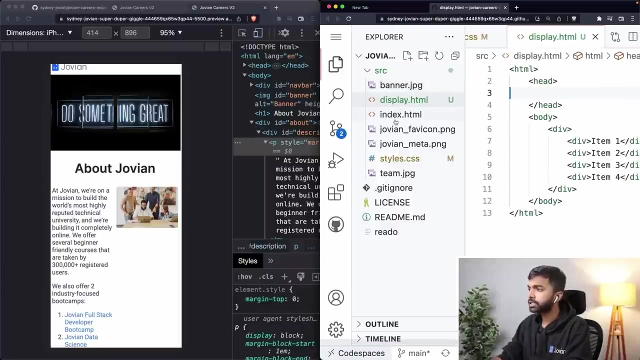 Okay, Body, and in the body, let me put in a bunch of divs. let's create a div called item one, item two, item three and item four. Okay, And let us open up this page using the live server. 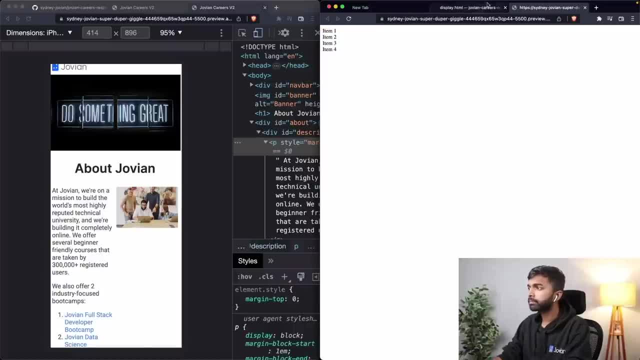 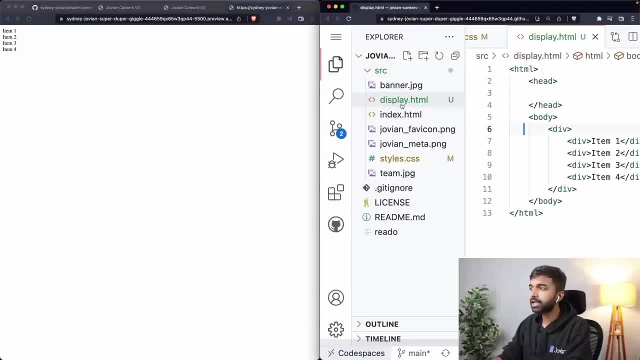 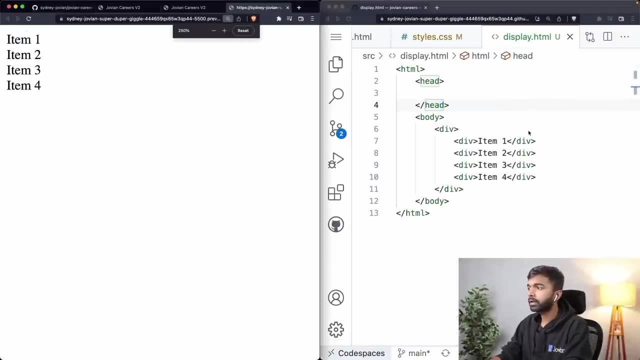 So let us right click and say open with live server And we'll open it up here. The way to open up any page in live server is by simply right clicking and selecting open with live server. Okay, And you can see that we have a bunch of these divs here and I'm just going to set the display property for each of these divs. 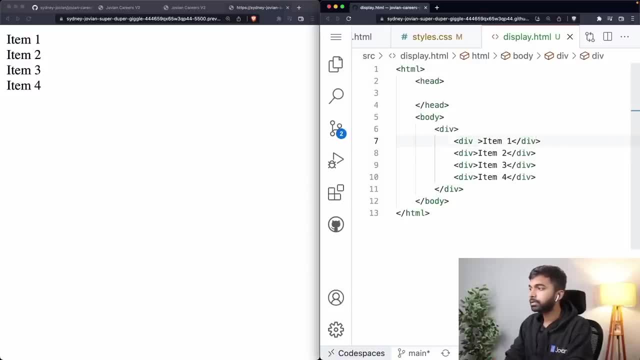 The first. I am going to set the display property for item one. Let me just give it the ID item one And let me give this the ID item two. Okay, Item two. Let's go ahead and give them item three and item four. 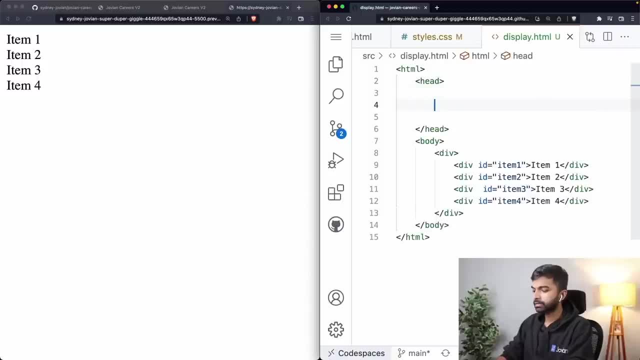 Yeah, So you have a bunch of items here and let us go ahead and set the display property for item one to display block And let's put that inside a tag. Okay, That is how we are. Okay, We can do a little bit of work on the display property. 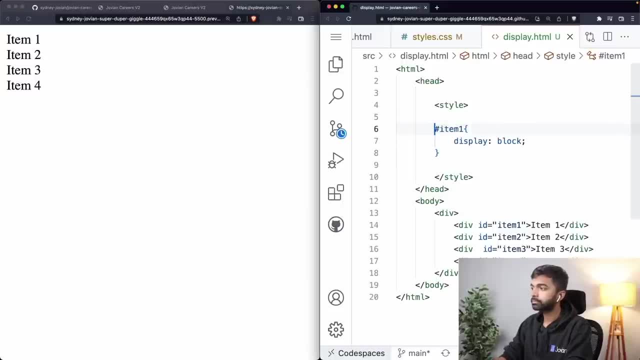 So here we have a dot entity here. This is the item one flag which I'm going to be applying CSS. So there is no change. when we set the display of item one to display block. What happens if we change the display of item one to display inline? let's actually add a border around item one so that we can get a better sense. 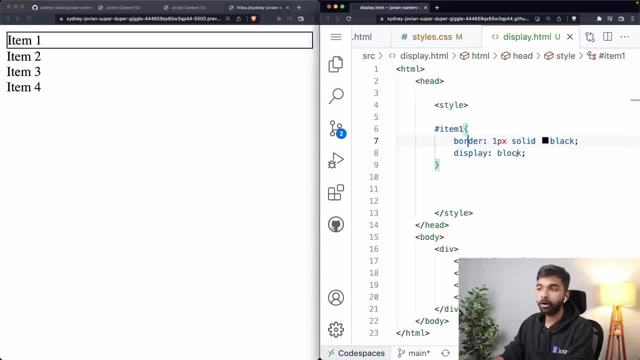 Yeah, You can see here that when you have display block, which is the default value, Yeah, item 1 takes up the entire width of the screen. Instead, if we set display inline, you can see that now item 1 does not take up the entire width of the screen and, in fact, 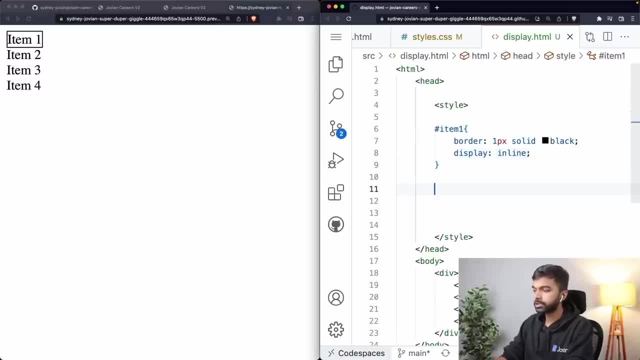 it will show up inline with other things that are also inline. So let me just go ahead and for item 2 as well, let me add a border: 1px solid red and let me set the display inline to inline as well, And you can see here that item 1 and item 2 both show up on. 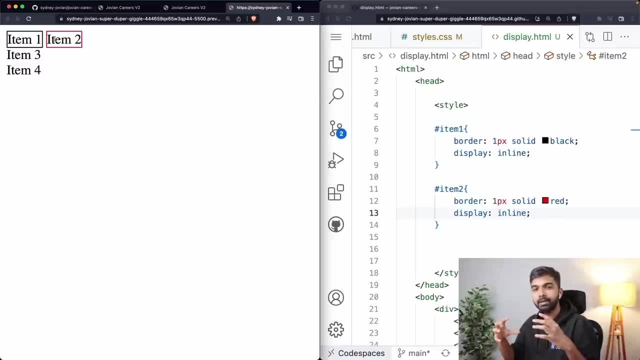 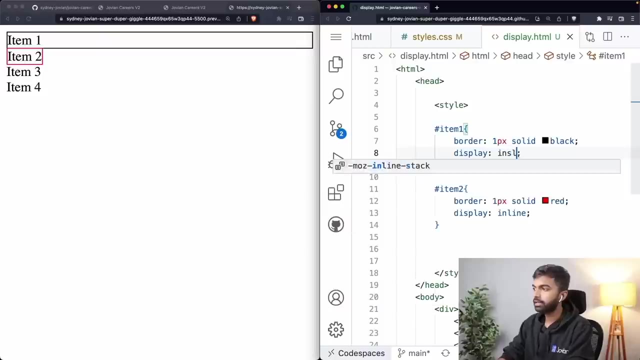 the same line because they are set to inline. So display inline does not take up the entire width and allows a particular div to get embedded inline within some text or within other inline items. But if either of these was block, you can see that that no longer is true, So that 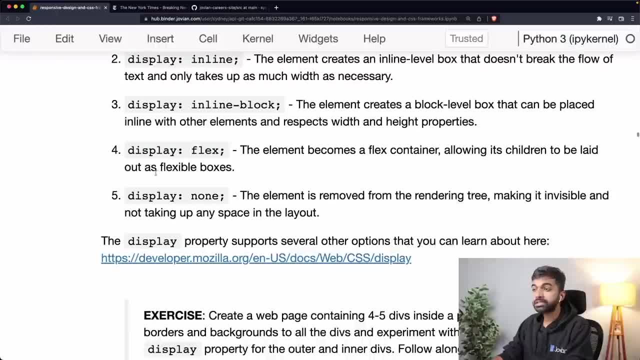 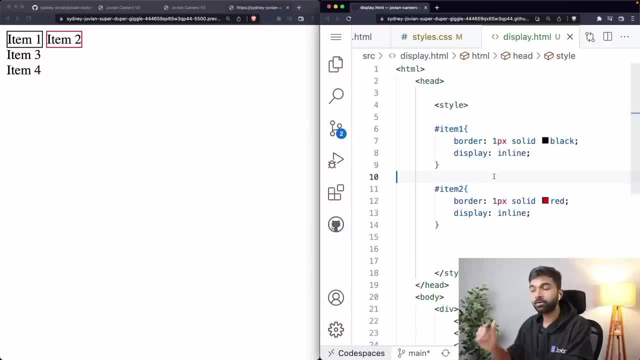 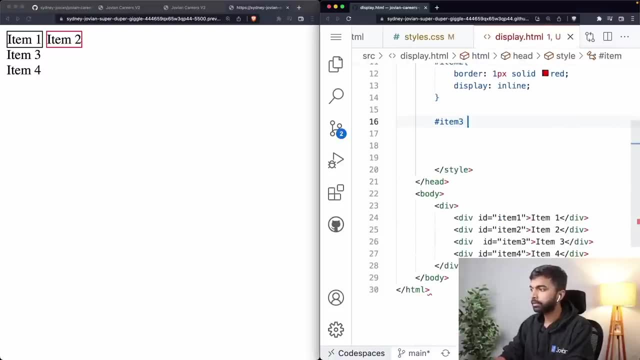 is display inline, and then there is something called display inline. This is a block which I will leave to you as an exercise, So I'll let you figure that out, what that does and how that's different from display inline. Then there is something called display none. I can say item 2 or item 3, display none. Now it just disappears. So 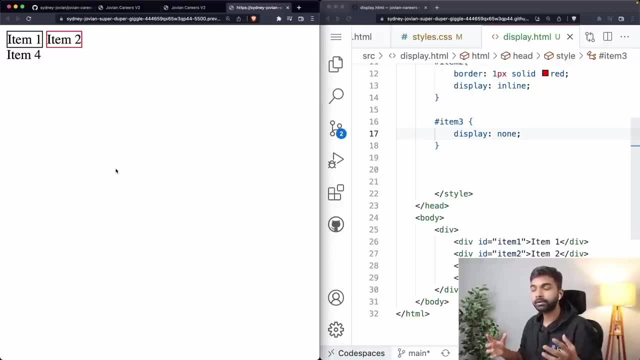 when you don't want to show a particular div- and we'll see an example of this later today- then you just said: display none. Now the final property that we are going to study, which is what triggers the flexbox layout, is the display flex property. So we're going to come back and we're going 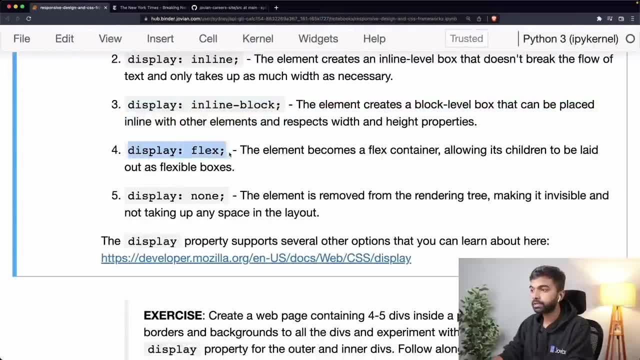 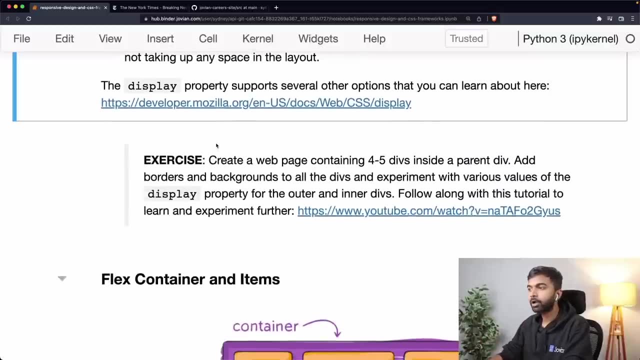 to take a closer look at the display. flex property is- which is what makes a particular div a flex container and allows its children to be laid out as flexible boxes- Very important. We're going to look at that in just a second. But there are also several other display options. 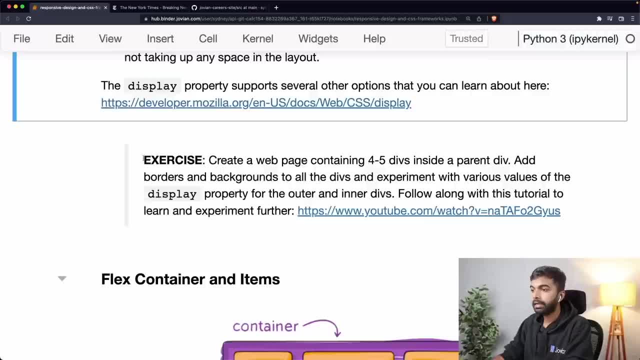 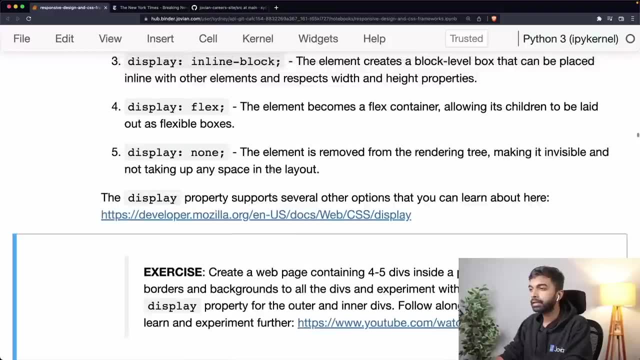 So I encourage you to check out the other display options as well, And I encourage you to also maybe try out this exercise, which goes into the various options that you have for the display property, But these are the most common ones that you'll use: display block, inline flex and possibly none. Okay. 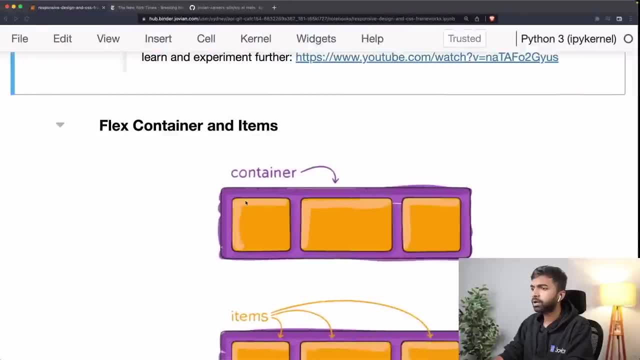 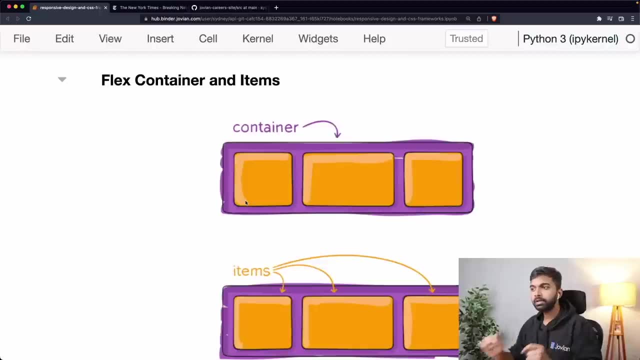 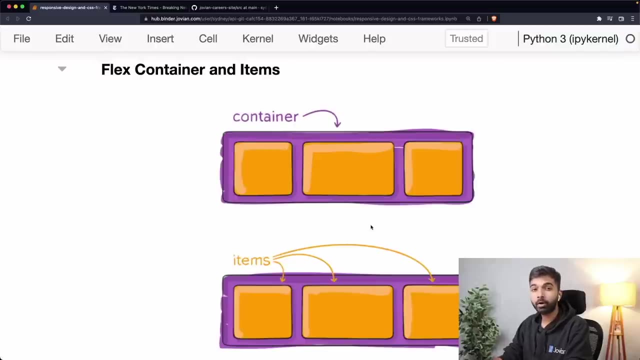 So with that, let's close this. let us talk about flexbox Now, the first key thing you want to understand about the flexbox layout is that it works with containers and items, So you always have an outer div which is a parent or a container. 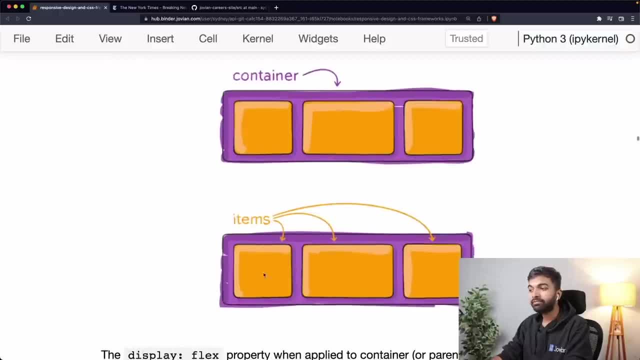 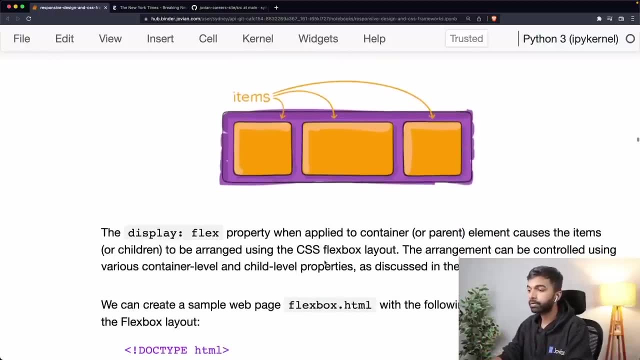 on which you set the display flex property, and then you have the items, and the items are then laid out in a flexible fashion based on a bunch of CSS properties to set the display flex property, when applied to a container or a parent component, causes the items or. 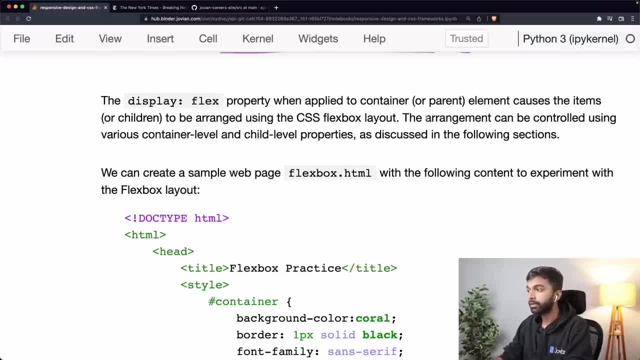 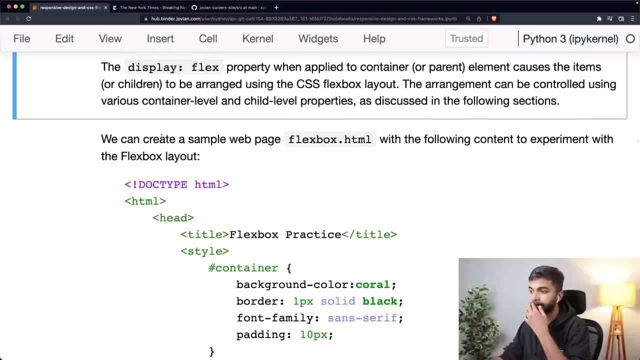 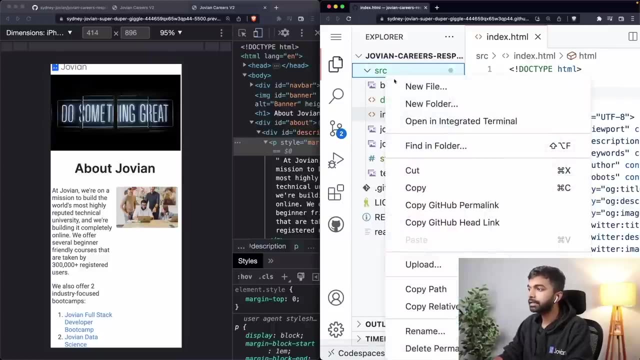 children will be arranged using the CSS flexbox layout, And the arrangement can be controlled using various container level and child level properties, as we will discuss in just a sec. So let's go ahead and create a new file called flexboxhtml. I'm going to right click here and create a new file called flexboxhtml. 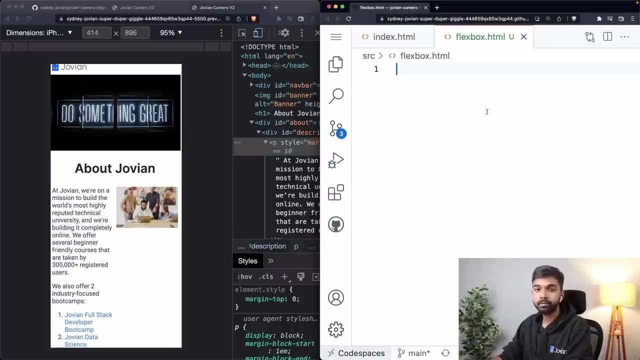 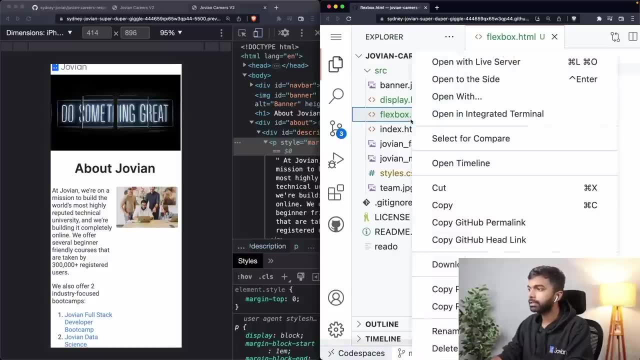 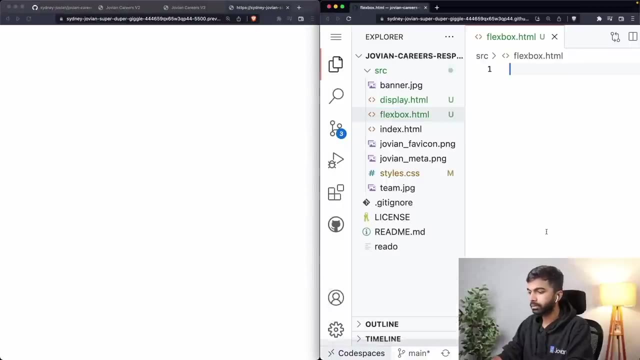 Into this file, flexboxhtml. I'm going to add a bunch of HTML and CSS code to set things up. Let me also open it up quickly in the live preview. So open with live server. Let us open it up over here And let us see. 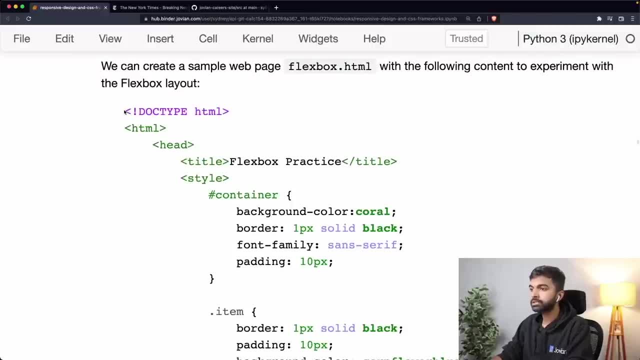 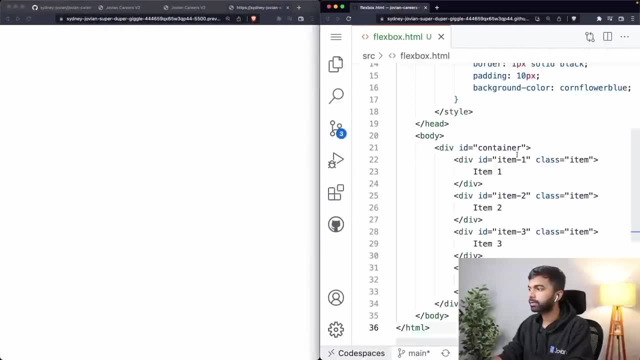 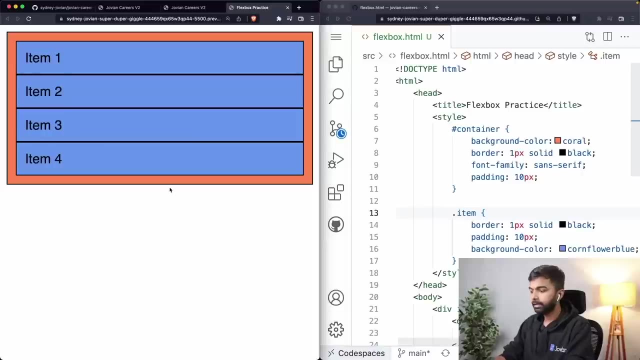 Let us come back. Let us set up the code for this. I'm just going to copy this code and paste it in here, And we'll just walk through the code and then start studying a bunch of Okay. so this is what our content currently looks like. 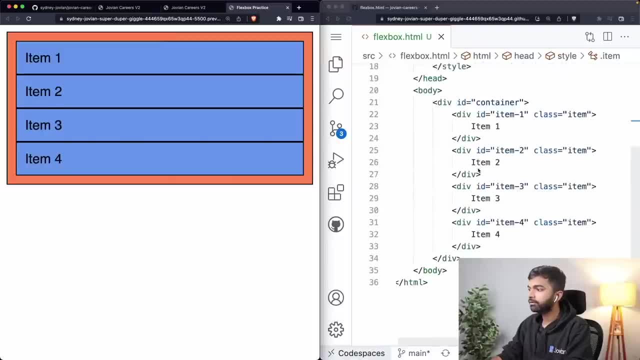 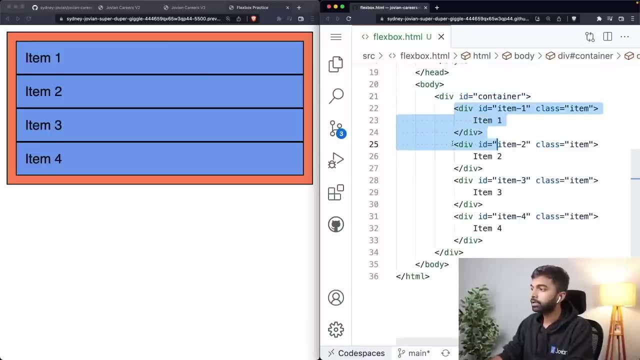 We have a box, We have a div, we have a div with the ID container over here And then inside that div we have four divs: One called items, One called item one, another called item two, another called item three and another called 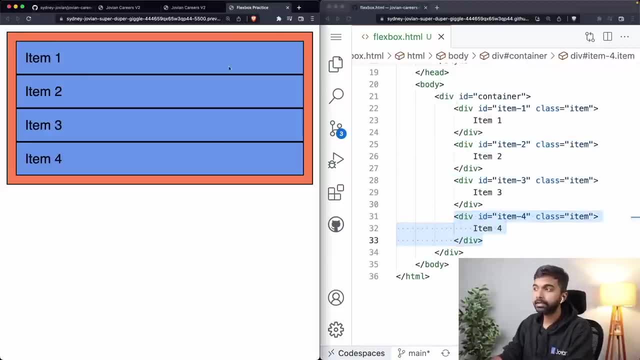 item four. So we have these. we have this container div. that's clear. The container div has four item divs And each item div has the ID item one, item two, item three, item four respectively, And all of the item divs have the class item. 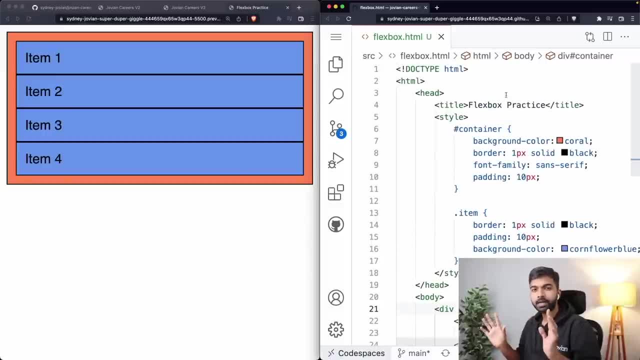 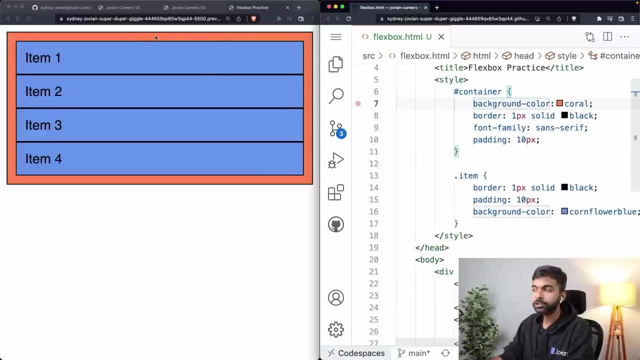 Okay, And let us look at the CSS. So so far we've not used flexbox flexbox at all. for the container, we have set a background color of coral. you can see that it has this orangish background color. 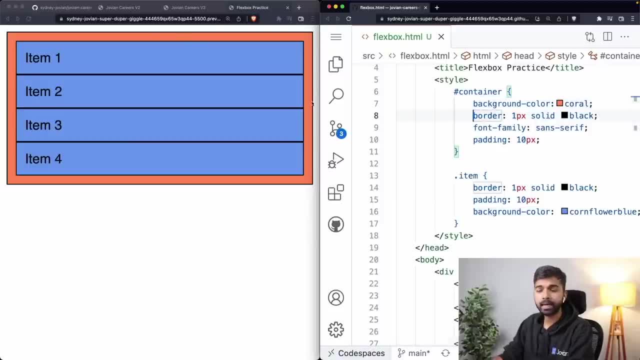 And then we've also given it a background- one pixel solid black background, a border of one pixel solid black. we have also just set a font family so that the font, the text, is a little easier to read. And finally we have given it a padding of 10 pixels. 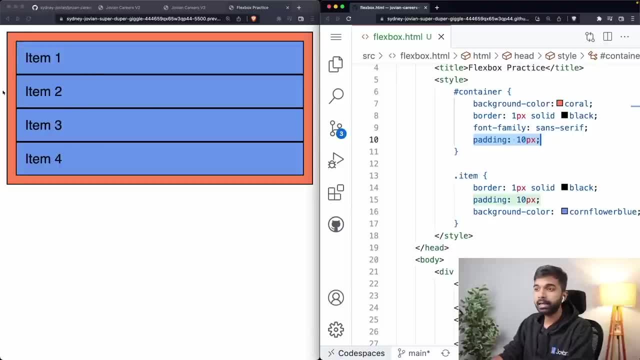 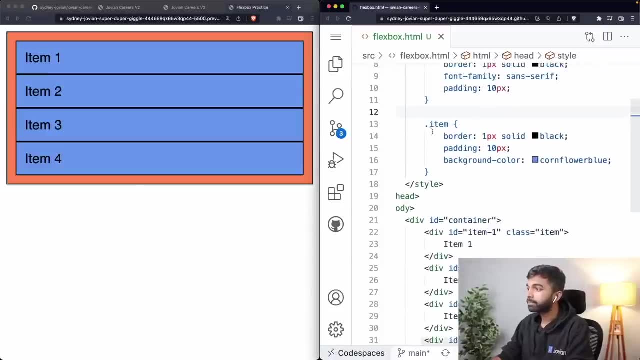 So you can see that there is a 10 pixel padding inside the border and then there is a content inside it. Okay, so far we've not modified the display property. then we have the item for each item And again this is a class. 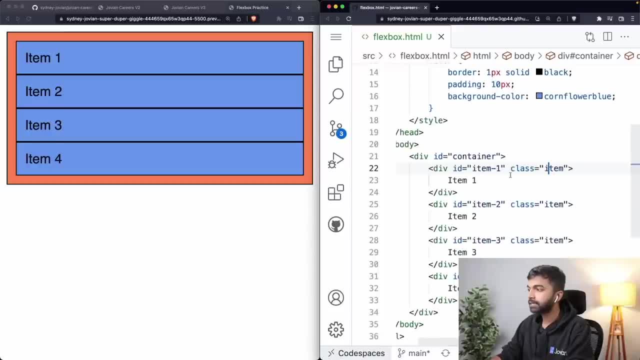 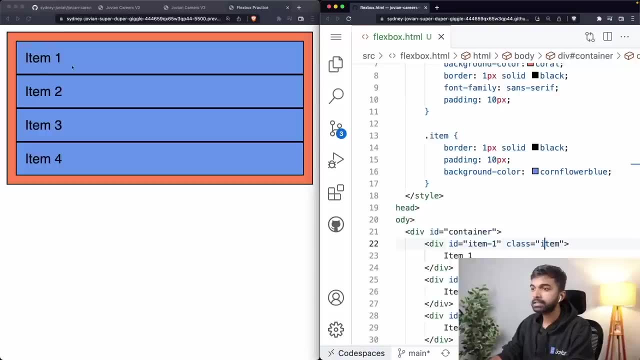 This is a class item, not individual items. So we have specified the class item for each item. we're not using the IDs just yet. we have again set a border of one pixel. we have set a padding So you can see that there is some space around the text. 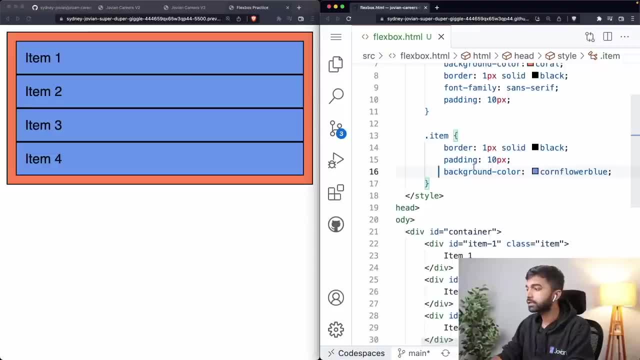 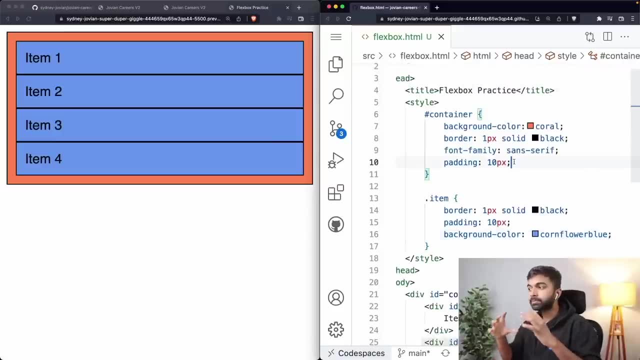 And finally, we've set a background of cornflower blue. that is the blue that you're seeing. Now let us slowly start turning this into a flex container. So always the flex display property is set on the container. So we say display flex. 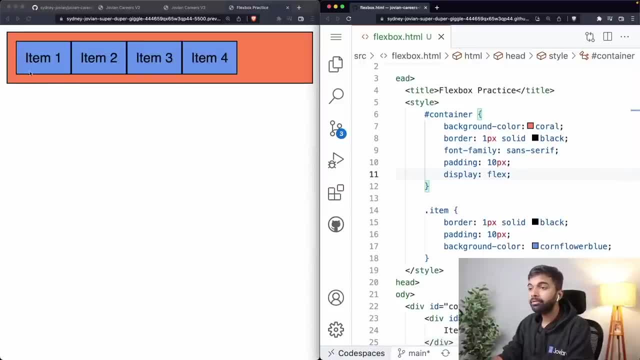 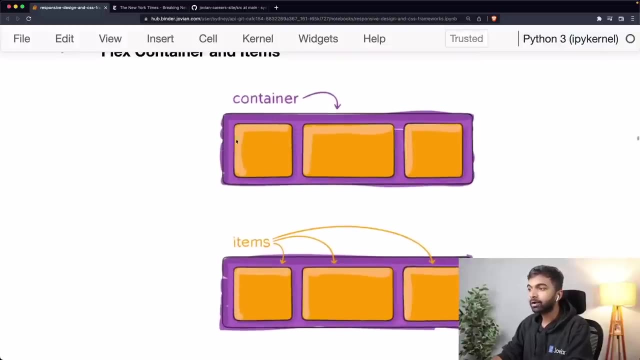 And I'm going to hit save. And now you can see suddenly that all the items are now laid out in a horizontal fashion. Okay, so you set the display property on the container. On the container, you set the display property and that causes the items to be laid out according. 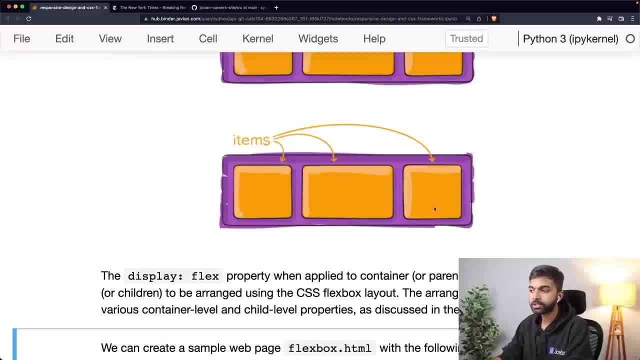 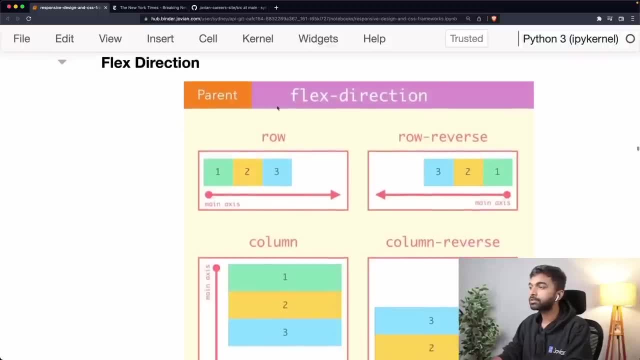 to the settings, the default settings of a flex box. Okay, So the first thing that we can change is the direction in which things are located. Things are laid out, and that is done using the flex direction property. The flex direction property has four values. 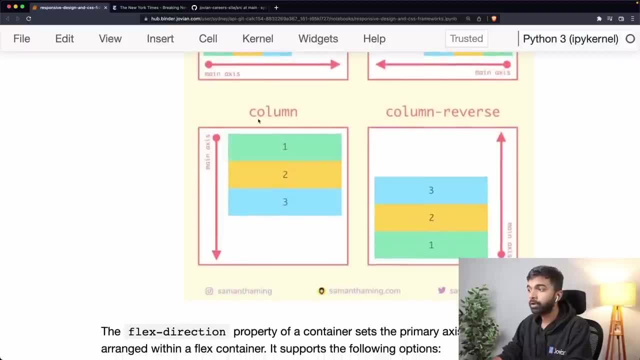 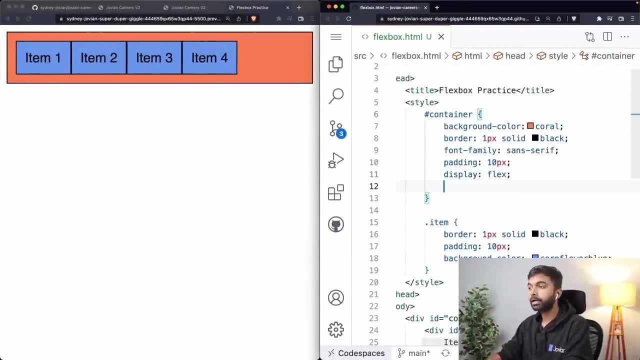 It has the row value as a row reverse value as the column value and the column reverse value. Okay, So let us take a look Again. all of these properties are first set on the container, And for each property we also have an example of whether it is set on the parent, which. 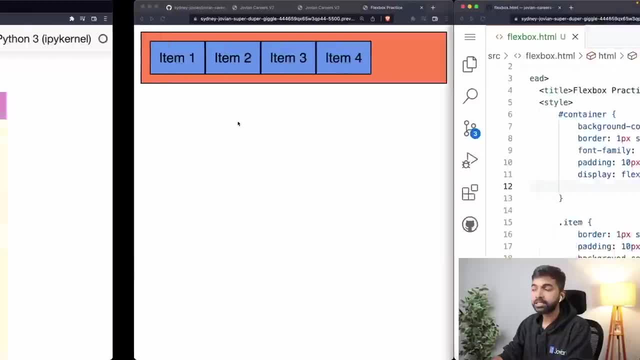 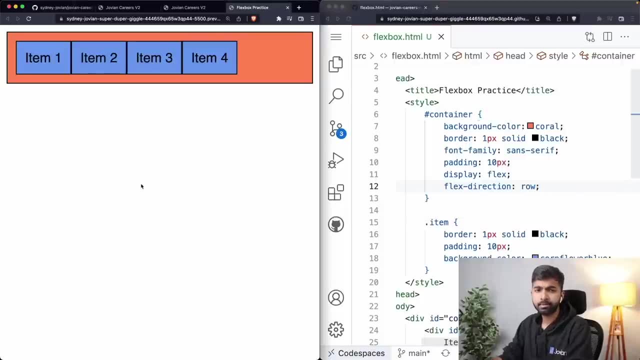 is the container or the child, So flex direction is specified in the parent. So we say flex direction row, And that doesn't change anything because the flex direction row is the default value. But we could also say flex direction row- reverse, And now you can see that the items are laid out not from left to right but from right. 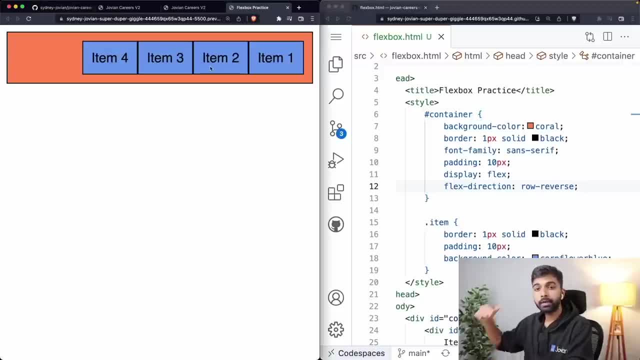 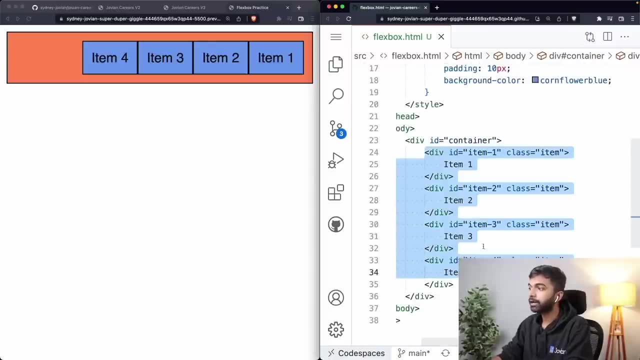 to left. So you have item one, item two, item three and item four laid out from right to left. Okay, They're still, logically, they're still in this order, but they're just laid out from light right to left, And this is where you can use flex box to maybe do some right to left layouts. 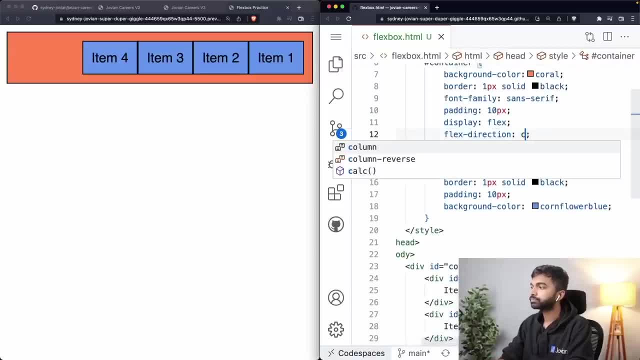 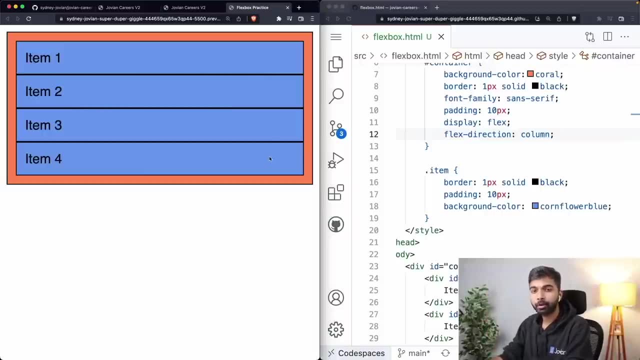 Okay, So let's check flex direction column. flex direction column, as you might expect, lays things out in a columnar format which is pretty similar to display block, but except you are setting that this is a column on the parent and on the container, not on individual. 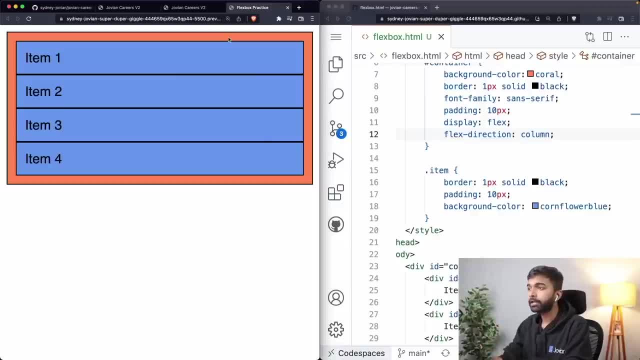 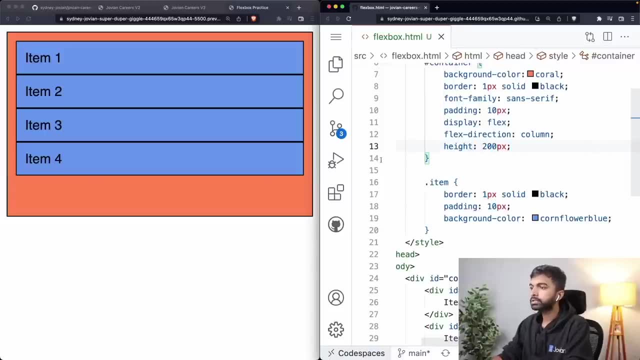 items. Okay, So flag, and of course you'll be able to set a lot of other properties as well. So this is flex direction column, and let me just increase the height of this so that I can show you clearly that the way things stack up is at the top. 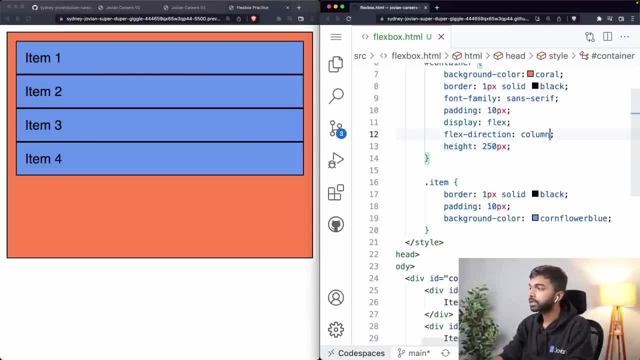 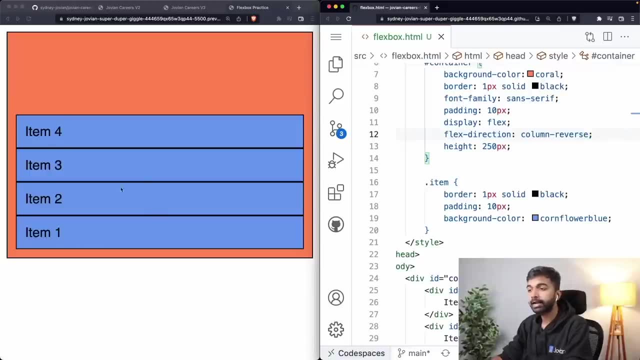 Okay, So flex direction column is top to bottom. You can also do flex direction column reverse and that will send things from the bottom to top. You can see item one above that, item two, item three and item four. So that is how you can lay things out. 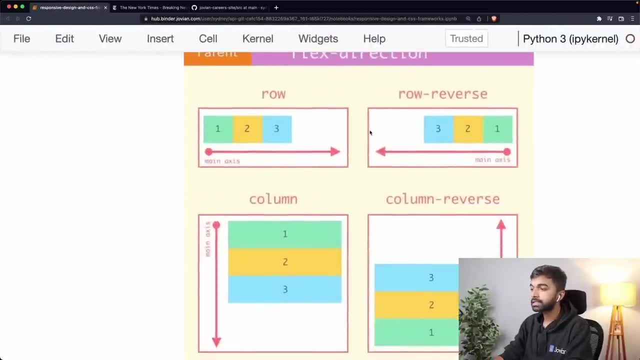 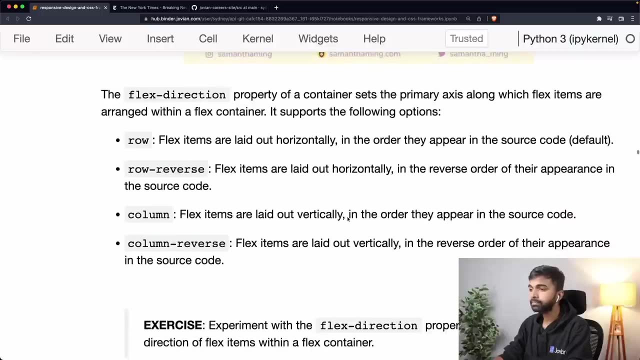 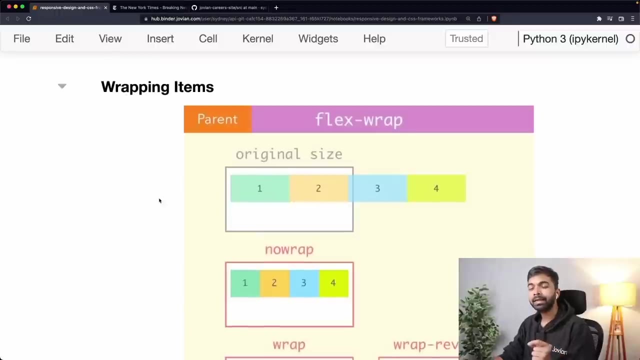 Flex direction row is left to right. Flex direction row reverse is right to left. column is top to bottom. reverse column reverses bottom to top. These are the four values you can set for the flex direction property and with flex box special specifically, I would highly recommend that you practice this, that you check out. 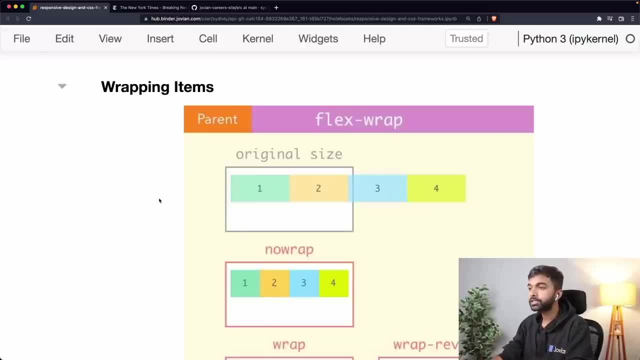 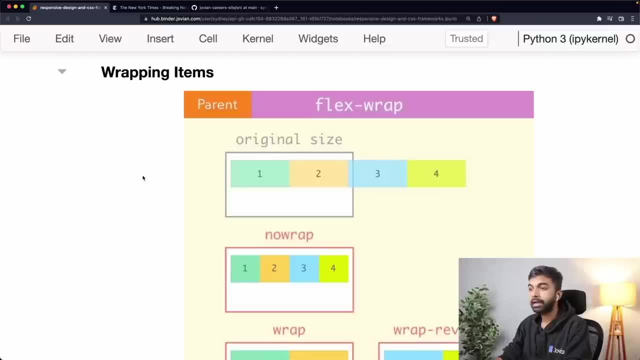 If you have a question- what happens if I do X- then just go ahead and try it out and maybe set proper heights and widths. You can use the starting code that we've provided here and experiment and understand and improve your understanding, Okay. 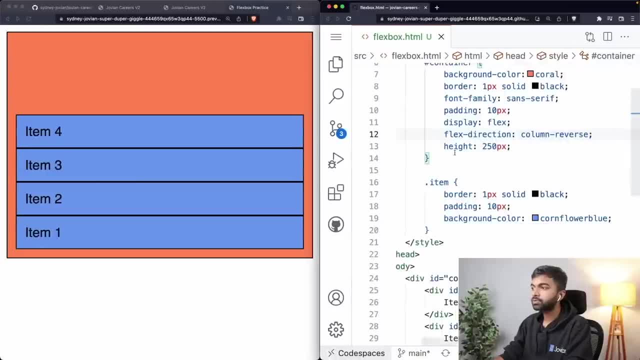 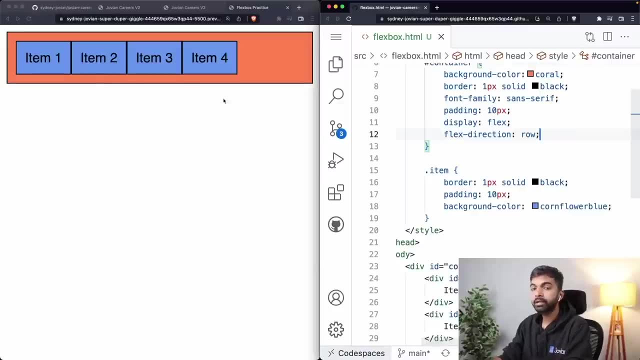 All right, So that's fine. Now the next thing is to check what happens If you have, maybe, data that is not going to fix within the given width of the container. So now we have a container, And now for this container we have a bunch of items, and all these items seem to be fitting. 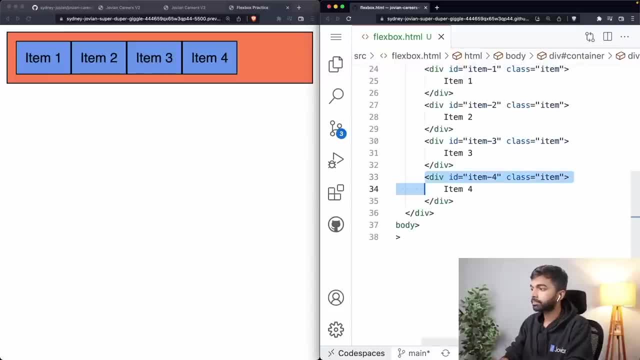 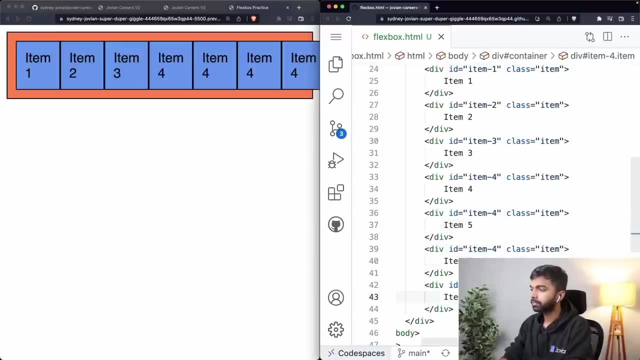 just fine. Well, what happens if we had more items? and say if we had item five, six, seven, right, So Okay, Okay, So item five, six, seven. clearly you can see what happens is first they try to compress. 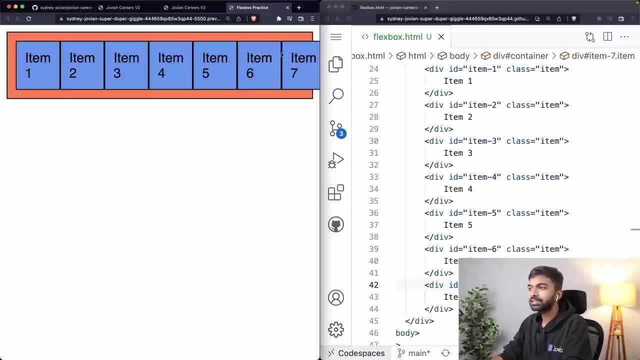 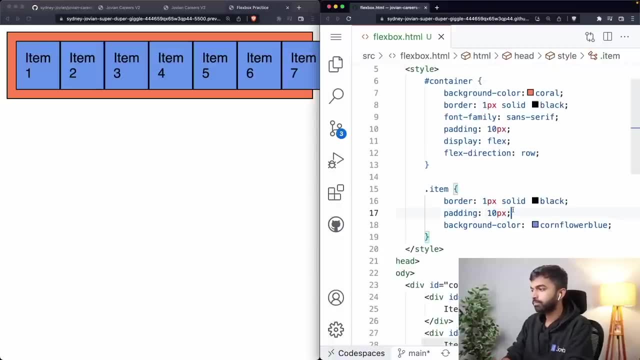 to fit within, but if they cannot go beyond a particular width, then they just go out. Then they just fall out. Now, when they do fall out, what do you do? Another another condition that could come up here is, let's say, our left and right padding. 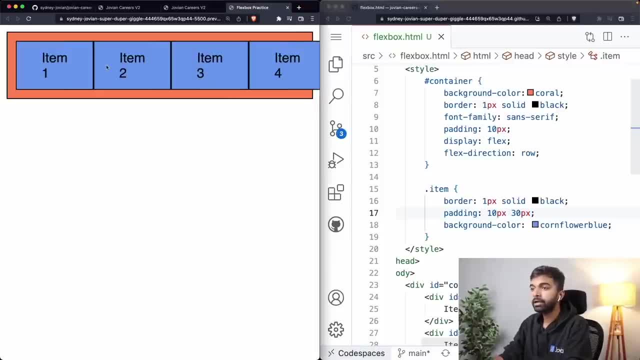 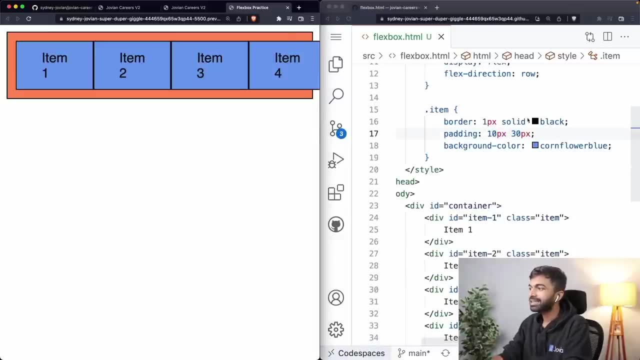 was actually higher. It specified a 30 pixel padding left and right. What are you going to do here Now? these, these all seem to be overflowing, These all seem to be going outside the box here, And that is where you can specify a flex wrap. 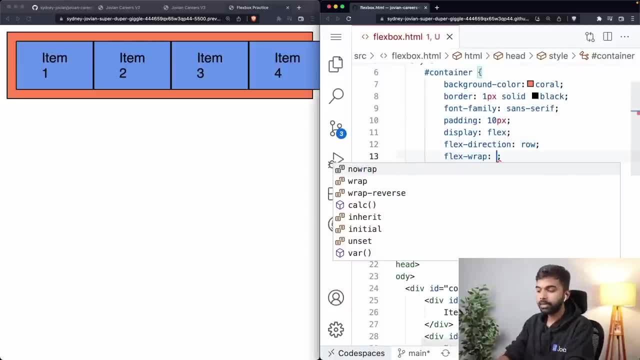 They can say flex wrap And the default value is no wrap. And again, this has to be set on the parent and specifies whether the container, whether the children, should be wrapped, which means they should go on the next line- or not. No wrap simply means that you want everything to show up on the same line, even if it exceeds. 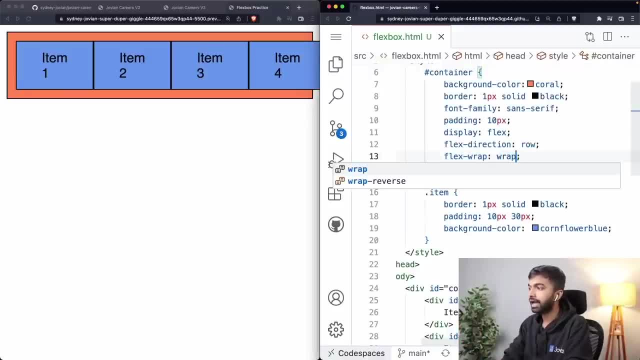 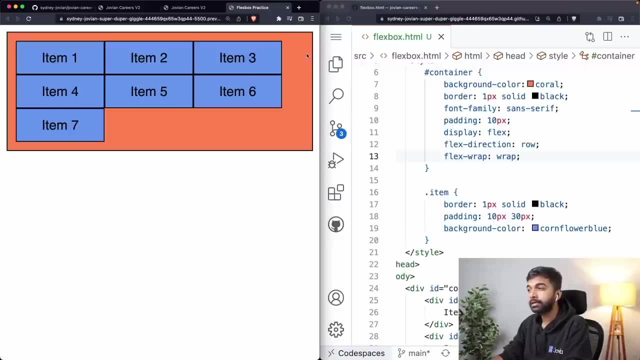 the width of the container. The other option is to say wrap, in which case this is what happens: It takes item one, two, three and then it when. as soon as it finds a tile element that cannot fit without exceeding the width of the container, it wraps onto the next line. 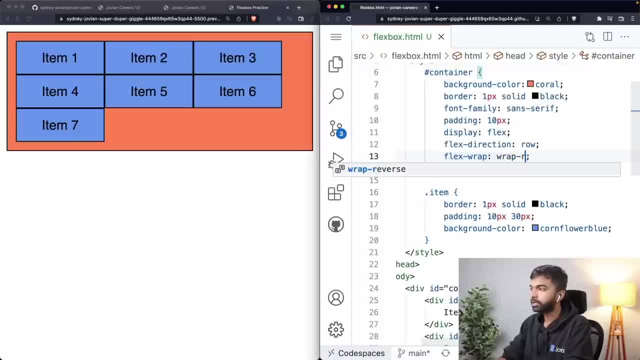 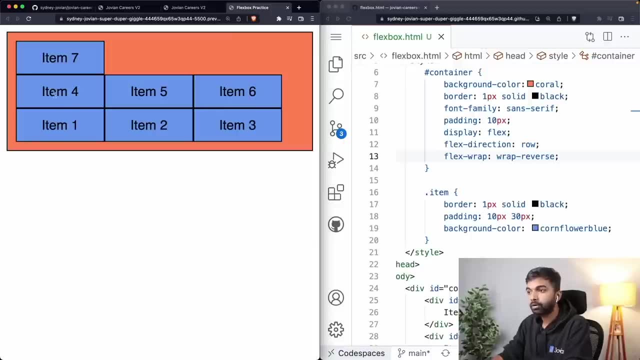 So we have five, six, seven. you can also do wrap reverse, And the idea here is that it wraps not onto the next line but onto the previous line, So you can say one, two, three, and then it goes four, five, six and seven. 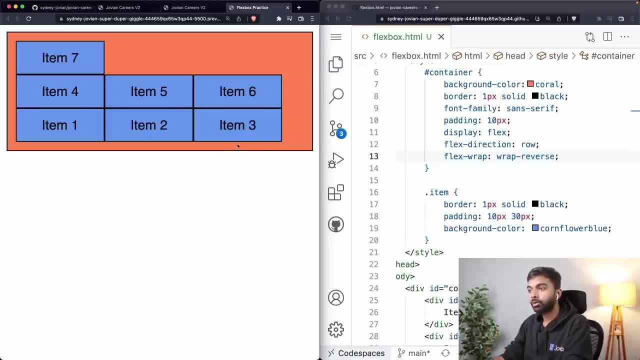 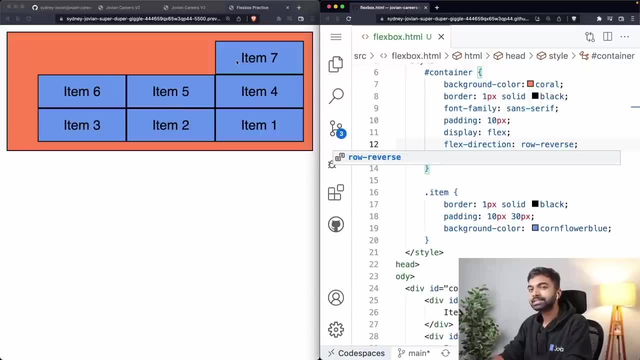 Okay, And notice this is different from row reverse. So if you did row reverse and you can check this out- it would now go one, two, three, four, five, six, seven. All right, Keep that in mind that you have a reversal on the row level. 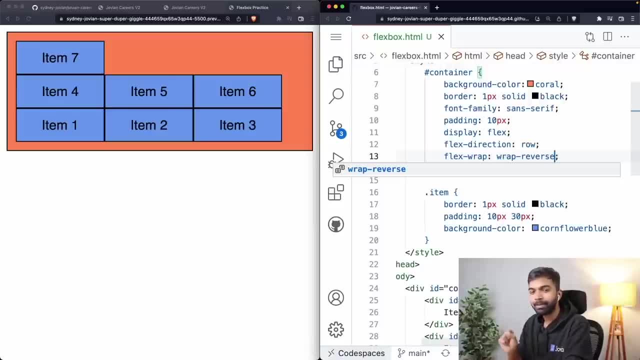 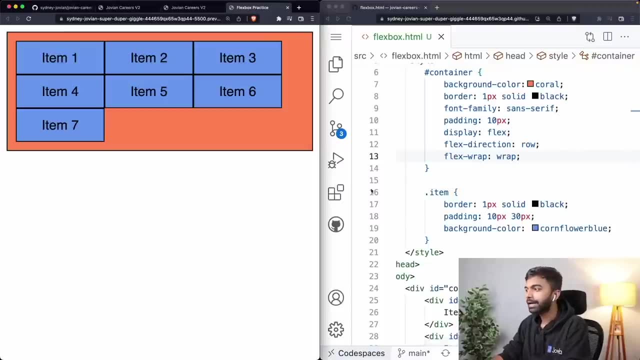 You have a reversal, possibly on the column level, and then you can do that reversal on the wrap level as well, whether you want the lines to go up or you want the lines to go down. Okay, So that is your. that is a flex wrap property. 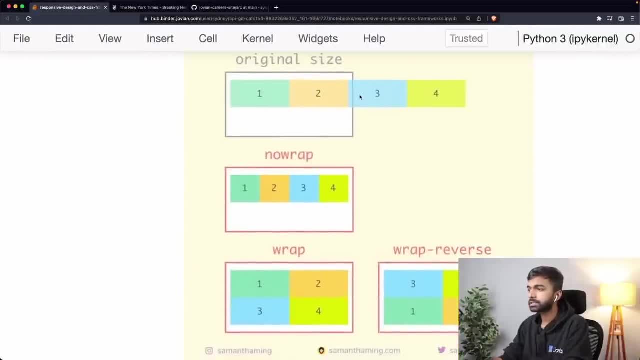 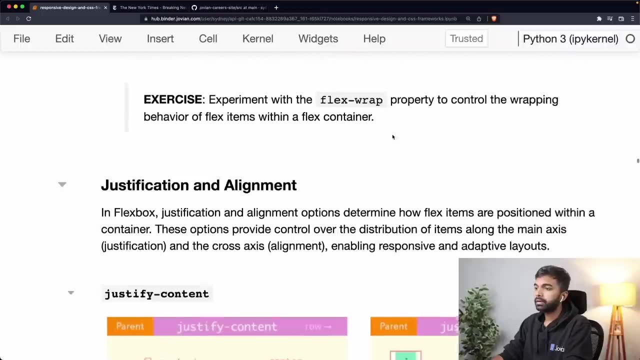 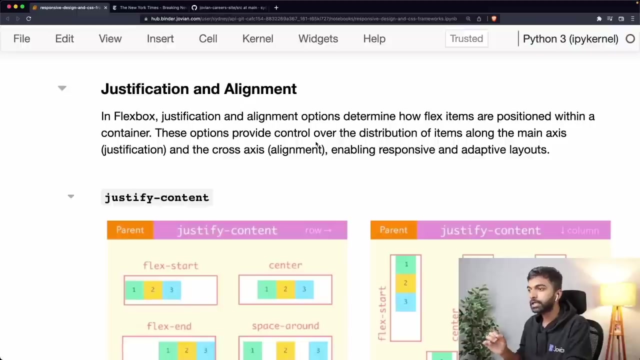 So you can, of course, just use no wrap, which is what just uses this, And then you have wrap and wrap, reverse. Okay, And experiment with this and you'll get a better understanding. Now the next set of properties, which are around justification and alignment, determine. 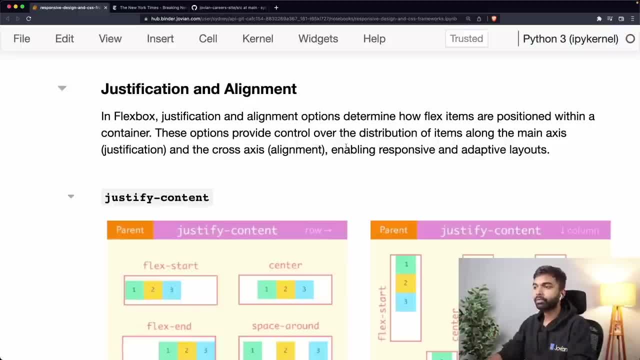 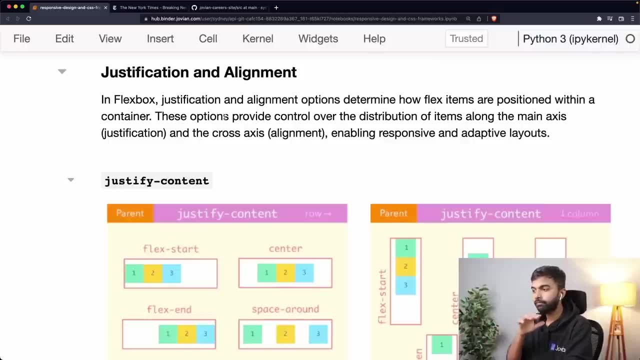 how flex items are positioned within a container. So these options provide control over the distribution of items along the main axis. The main axis, let's say, if it is a flex row, then the main axis is the horizontal axis and the secondary axis is the vertical axis. 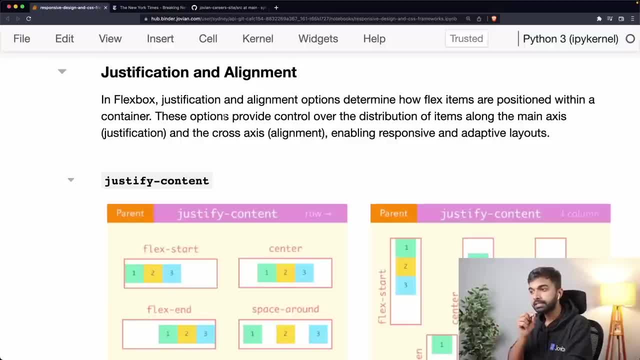 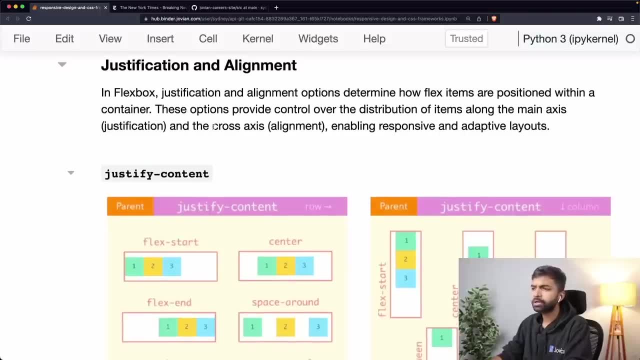 But if the flex direction is column, Then the main axis is a vertical axis and the secondary axis is a horizontal axis. Okay, So we'll just talk about it's also called the cross axis, So justification is controlled along the main axis. that is done using something called justify. 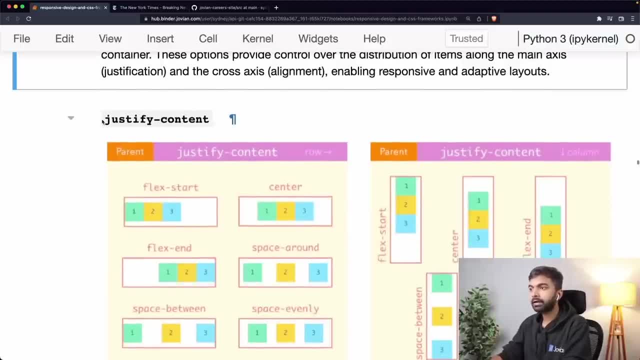 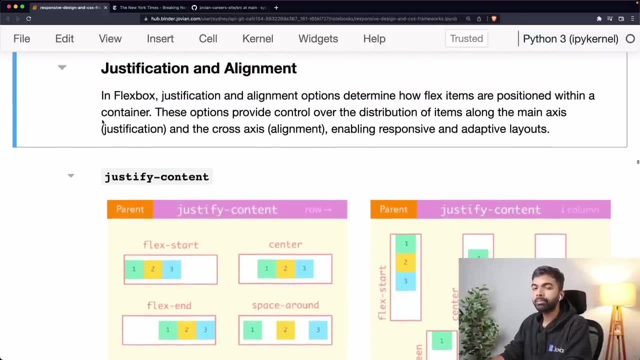 content and then alignment around is controlled along the cross axis. Okay, And I know this seems confusing. This is probably the most confusing part of flex box, but with some practice you'll get used to it. Let's look at justify content. 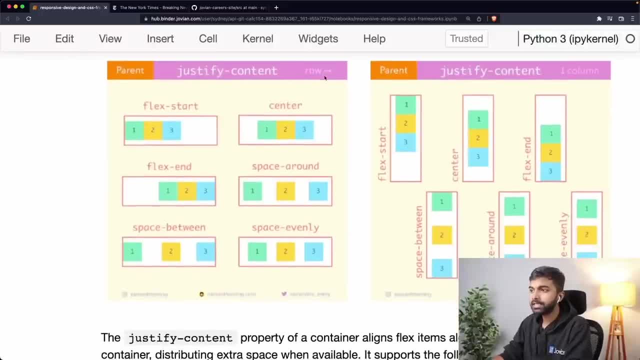 Now here is how justify content works. Let's say you have a flex container with flex direction row And on that container if you said justify content to flex start, then things will simply show up from left to right. If you said justify content to center, then the items will still show left to right. but 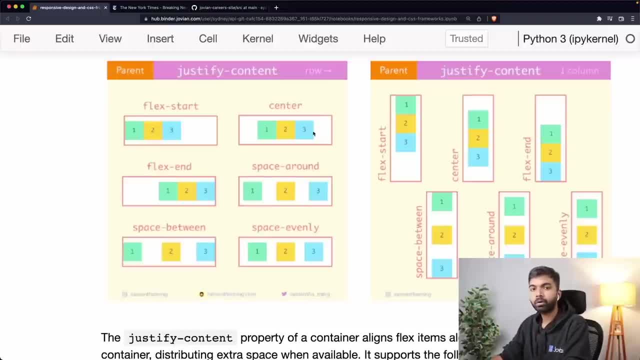 they will be centered on the horizontal axis or on the main axis, Right. So what that means is that all the items will be shown and then space will be added on the left and right. On the other hand, if you set flex end as justify content, then the items will just. 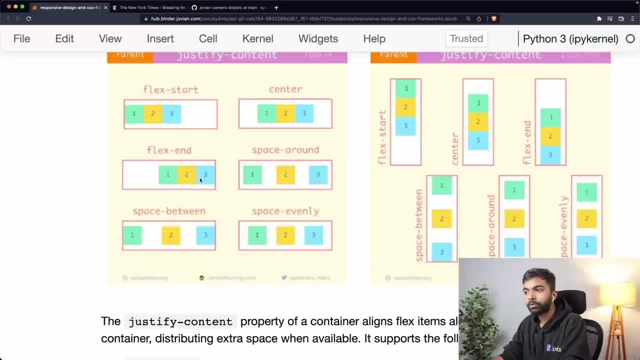 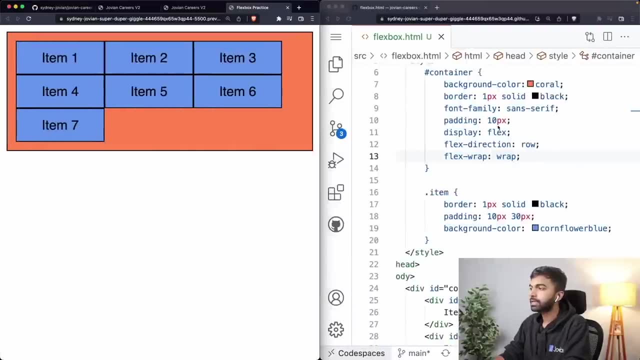 stick to the right. You notice they're still rendered left to right- one, two, three- but they are now sticking to the right side instead of the left side, And similarly, we have a bunch of other options as well. So let's take a look. 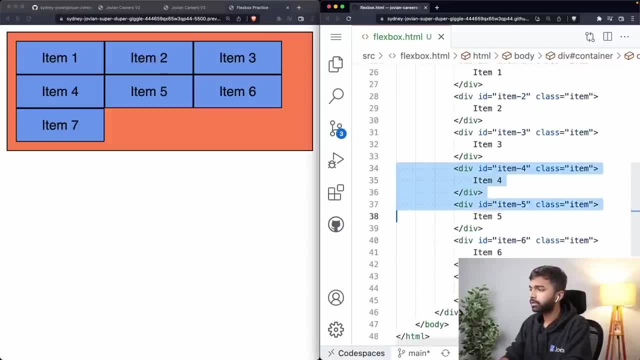 Let's get rid of some of these other items. So let's get rid of item four, five and four, five, six and seven, or just let's get rid of items five, six and seven. So I'm just commenting. 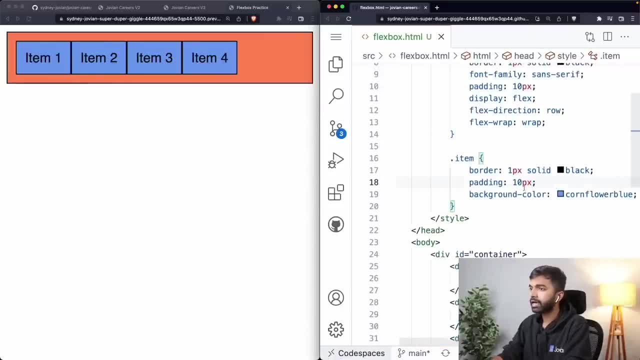 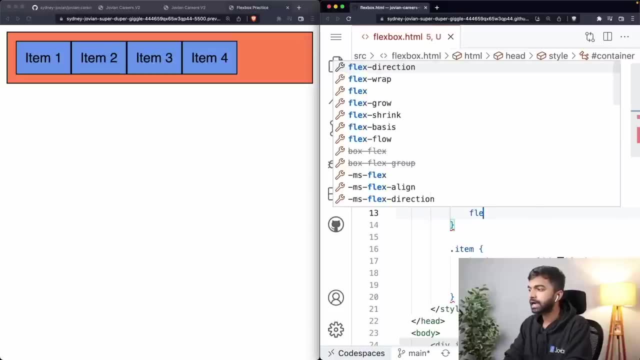 I'm just commenting them out and let us reduce the padding, the horizontal padding, for each item. So this is how they look right now. Now I can get rid of the wrapping for now as well. Now let me just add: justify content. 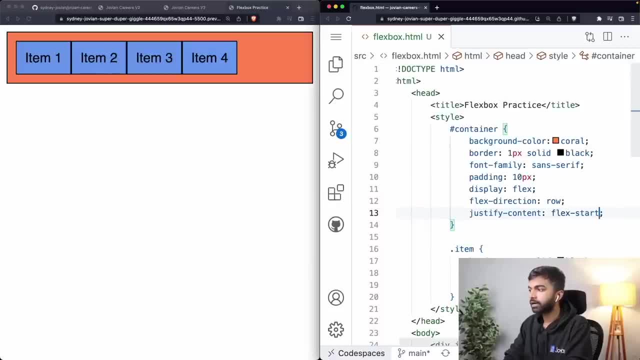 And again it's on the parent and let me say: flex, start. That's where they are. They're currently sticking to the start, which is the left right. It's not saying left, It's saying start, because if I had row reverse, then they would stick to the right. 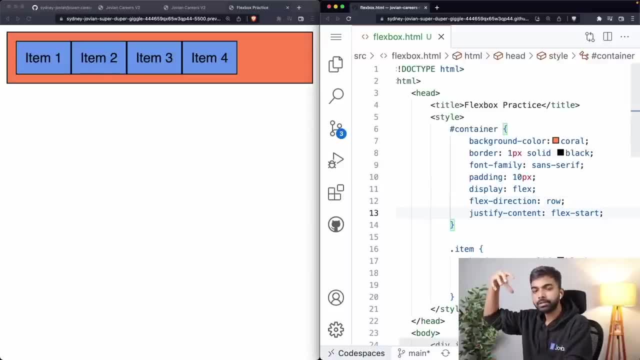 And if I had column they would stick to the top. So it just started: Start of the axis, whatever be the main axis, And now I could say: justify content center. Now you can see that they're still laid out left to right, but now they're placed at the 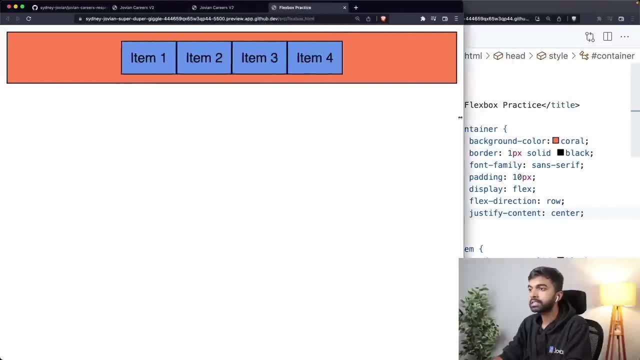 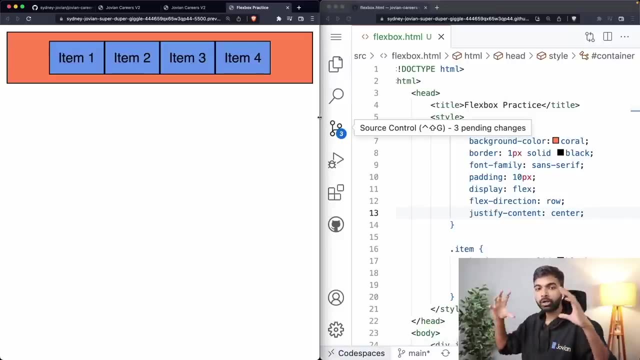 center And as I changed the width of the screen, you can see that they still remain right in the center. So anytime you want to horizontally center content within the page, just put an outer div. You can use the display flex and then put in an inner div and give the outer div justify. 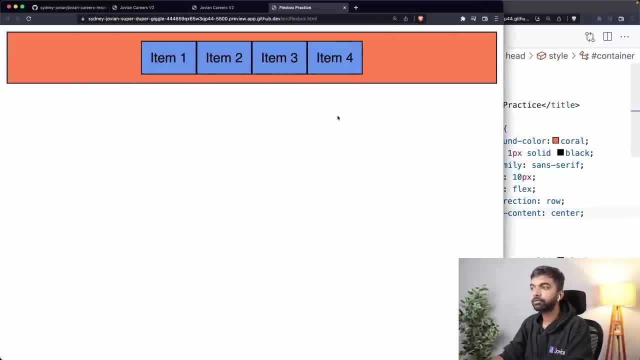 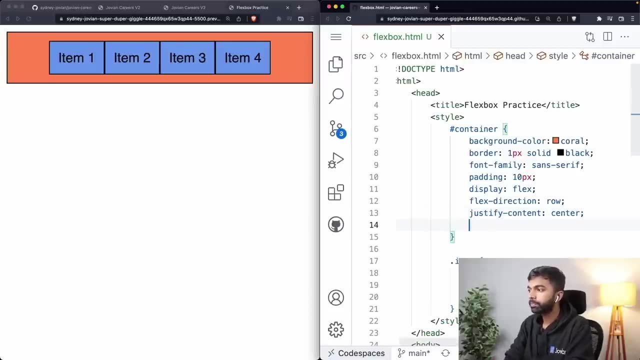 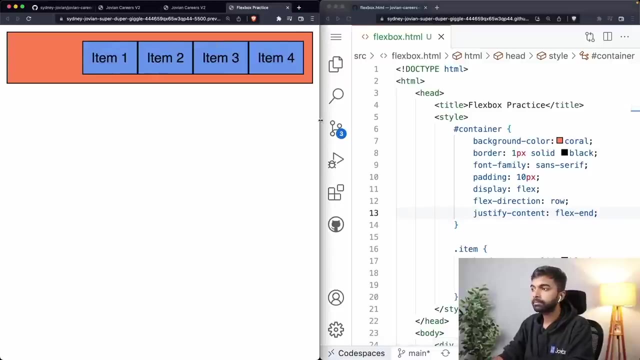 content center And that is going to horizontally center bunch of content on the page. very straightforward, Okay. Next let us now do justify content flex end. Now you can see that they are laid out at the end, So I modify. then there's another thing you can use. 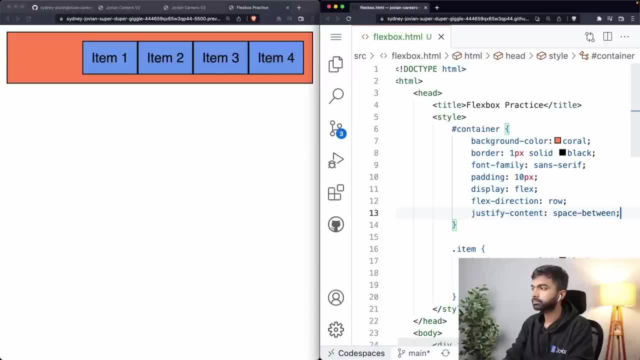 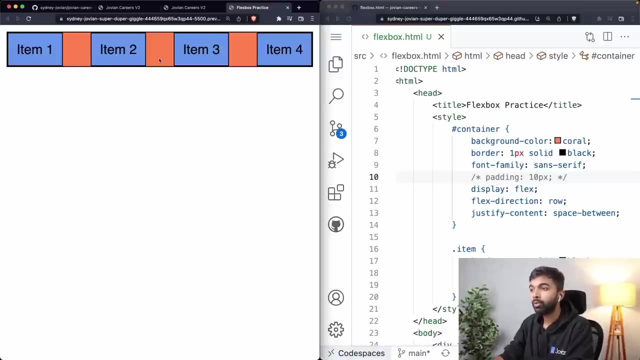 You can use. You can use space between. now, what space between does is: there is, of course, this padding for now. Let me just get rid of this padding so that we can have a better understanding of the space. So when you use space between, then faces added between each item and they are laid out from. 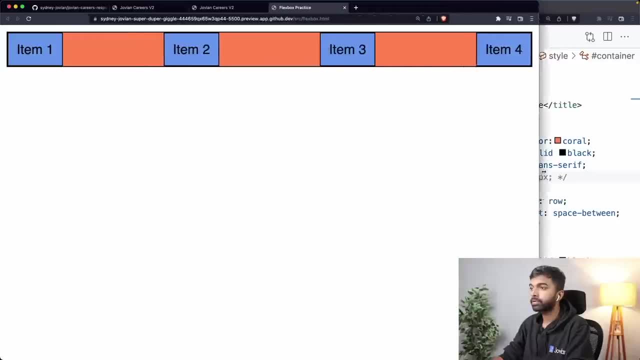 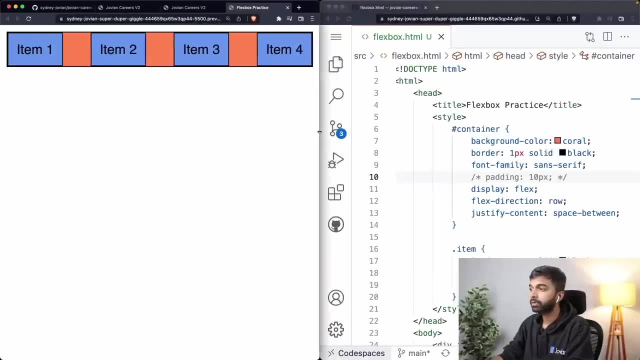 the left to the right with equal space between them, and see here that as I change the size of the page, this is added or removed between. All space is equal. Okay, Then you have face around. a space around is similar to space between, but what you do 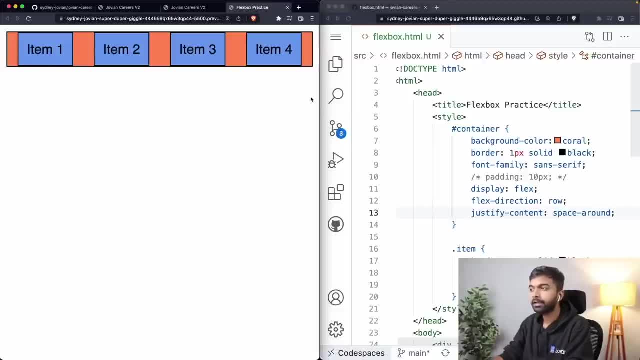 is, you take half of the space between and then you add it on the left and the right end as well. Okay, So that is what space around looks like. You can see visually that this space is about half of this space, and that is why I removed. 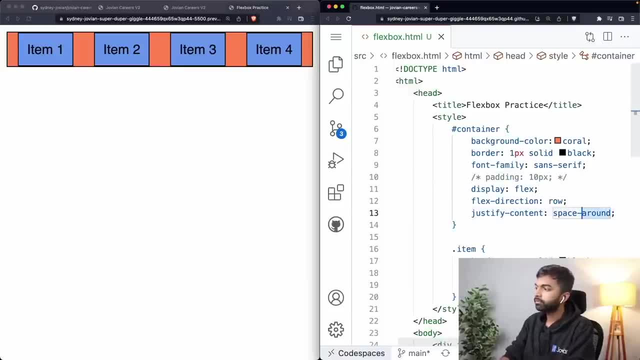 the padding for now, just so that we could clearly see these effects. Finally there is. Finally there is something called space evenly. a space evenly, as you can guess. what it's doing is it's going to add the same amount of space on the left edge, on the right edge. 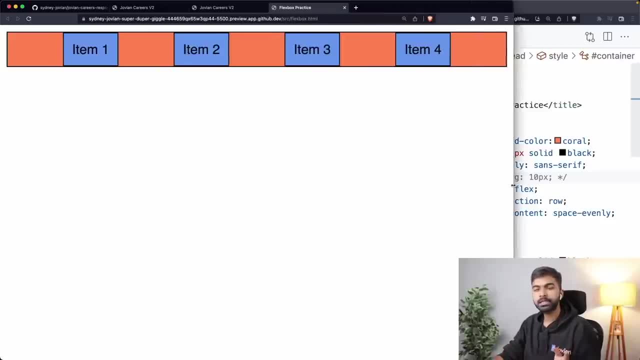 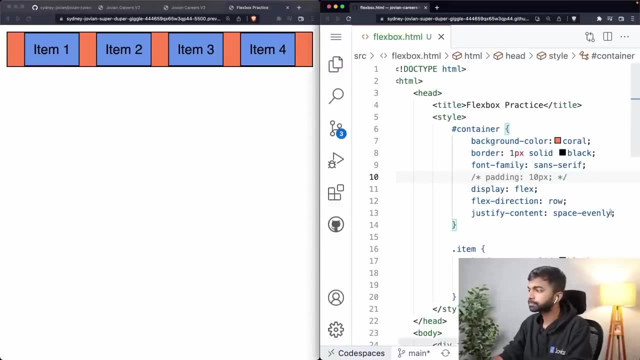 and between items. So slight differences between space, between space around a space, evenly depending on the use case. you can use one of these or just do something else altogether. Okay, But for now let me bring that back to next art, and we can also see this effect on a flex. 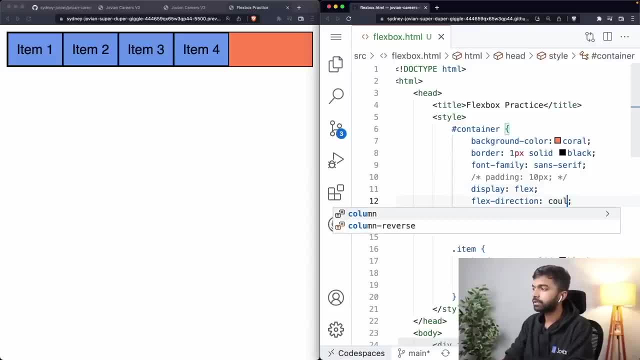 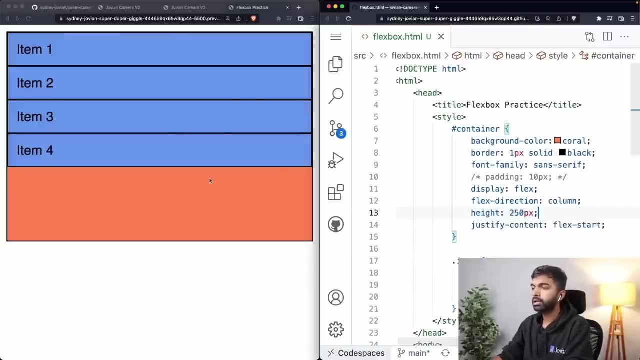 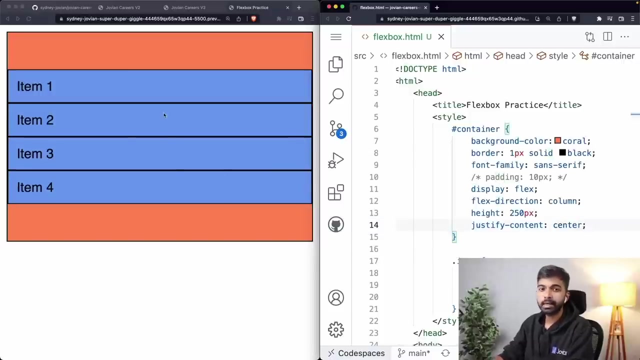 direction column. So let's say we have the direction column and let's say we have a height of 250 PX. here You can see that these are now laid out from the top. I can do flex end, Of course. I can then do flex enter and they are now centered. 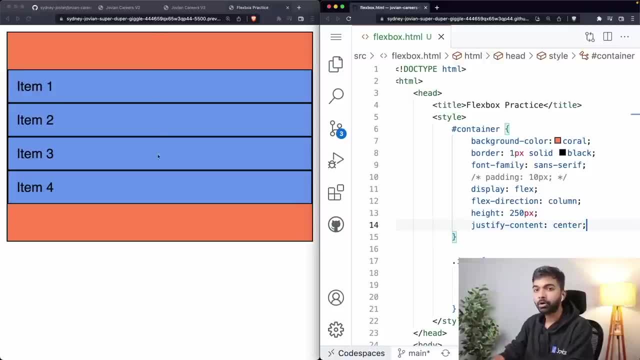 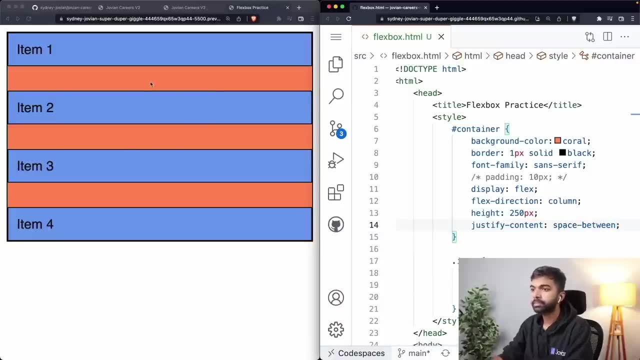 So now the main axis is the vertical axis And in fact it starts from the top. So the start is the top, end is the bottom, And I can do things like space around, space between as well. So this is space between. that is flex direction column. 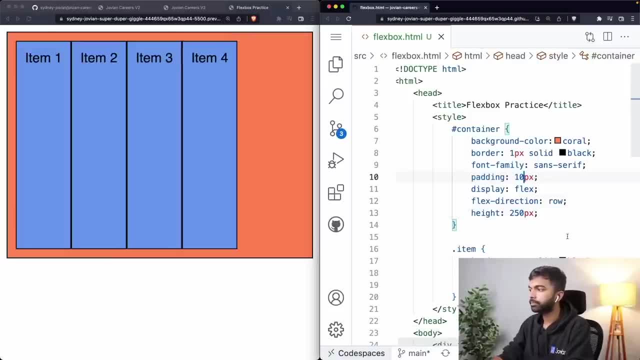 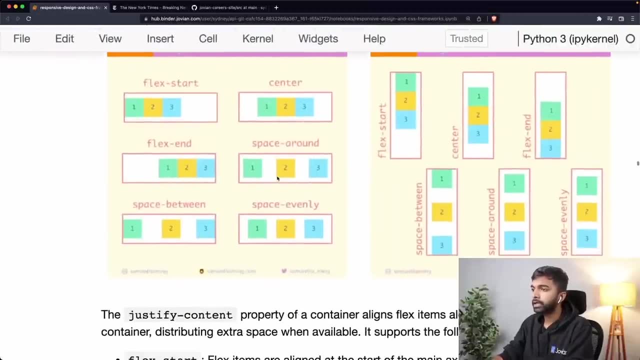 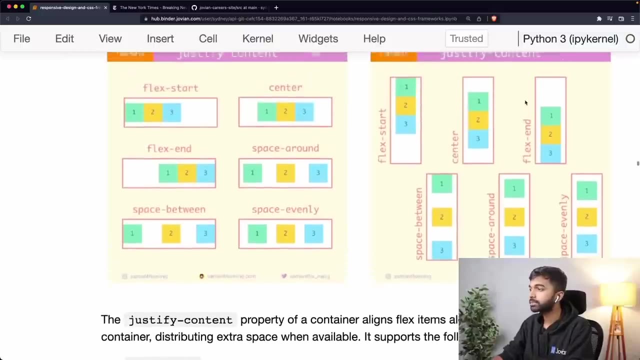 So all of these properties work for flex direction, row and column. get rid of that height, All right. So that is justify content like start, center and space around, space between and space evenly, And the same thing works for the column as well. 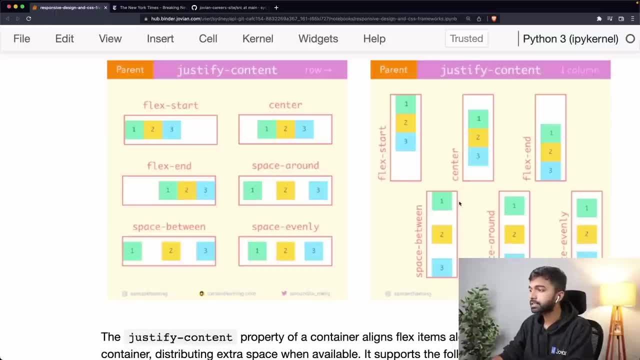 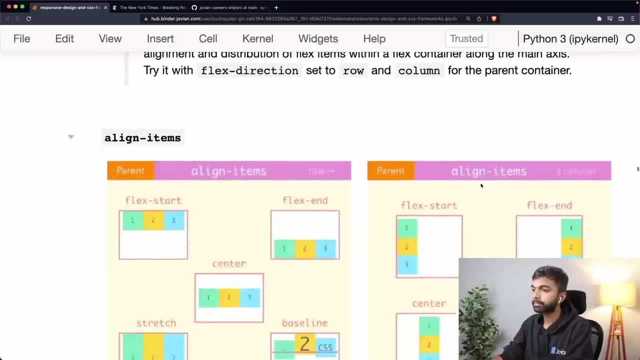 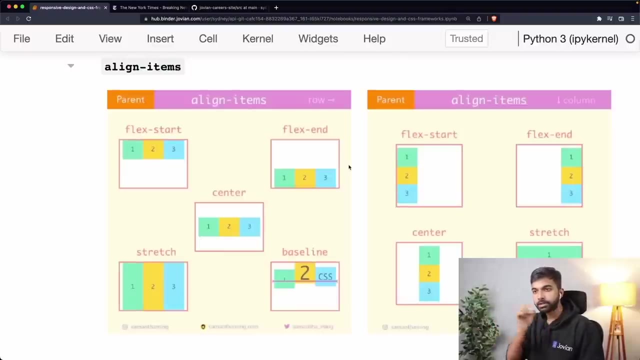 When you have a flex direction column. Okay, This is how the justify content values look. very powerful property. You will be using this a lot to create more complex layouts. Then we have aligned items. So justify content was along the main axis. So for flex row it was along the horizontal axis. for flex column: 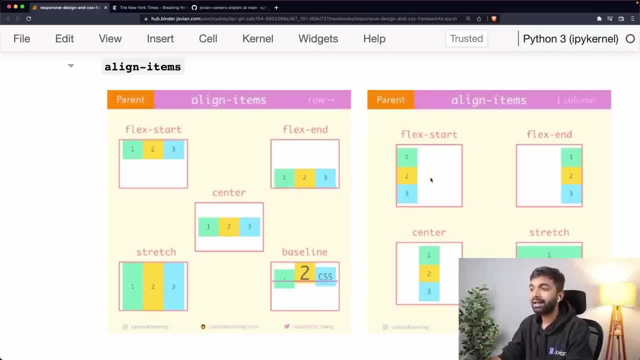 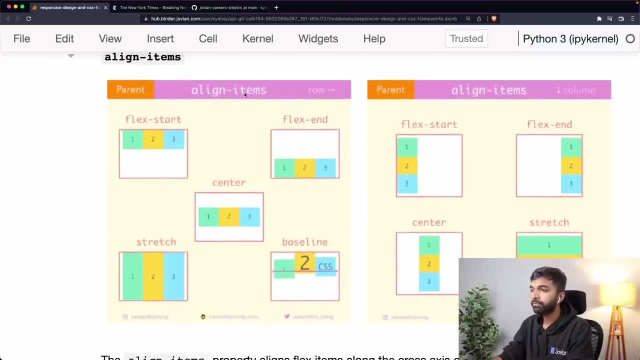 It's around the vertical axis. Align items is used to align things along the cross axis. Okay, So here is what that means. Let's say you have aligned items on your setting. Align items It means on a parent where the flex direction is row. 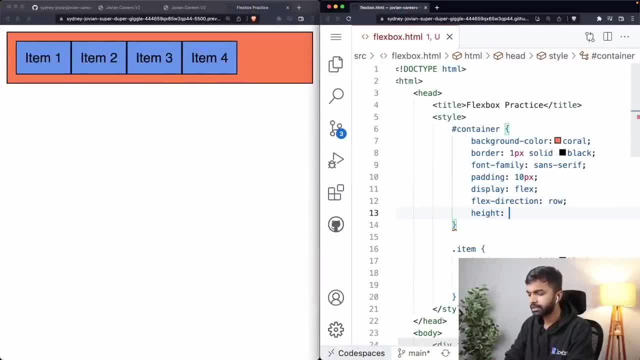 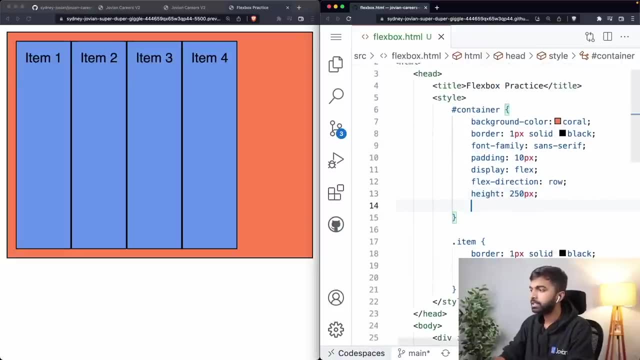 Let's look at an example of this. Let's just see this slide. Let's set the height to 250 pixels again. Okay, So the flex direction is row and I want to set the align items property. The default value is stretch. 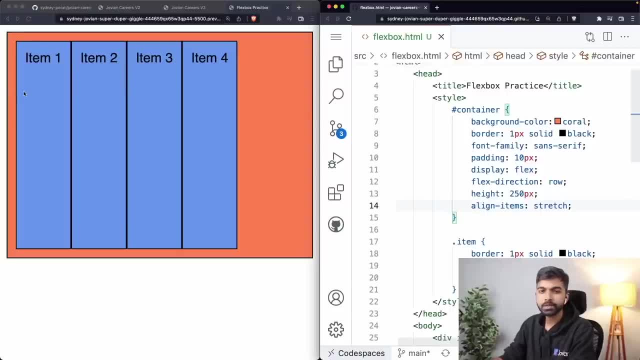 And you can see that as I increase the height of this div from whatever was the default height to 250 pixels, everything stretched, all of these inner divs, All of these Child divs, they automatically stretch to take up the full height or the full space. 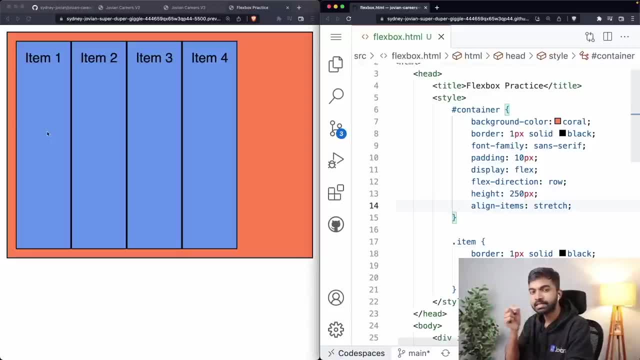 along the cross axis, which is the vertical axis, because the main axis is the horizontal axis. But I could also do flex start, So align items, flex start, So now along the cross axis or along the vertical axis, things are sticking to the start. 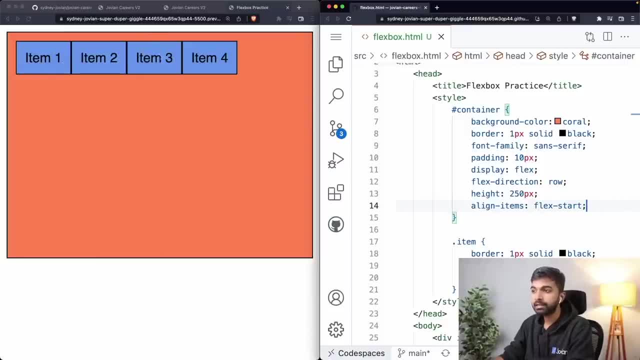 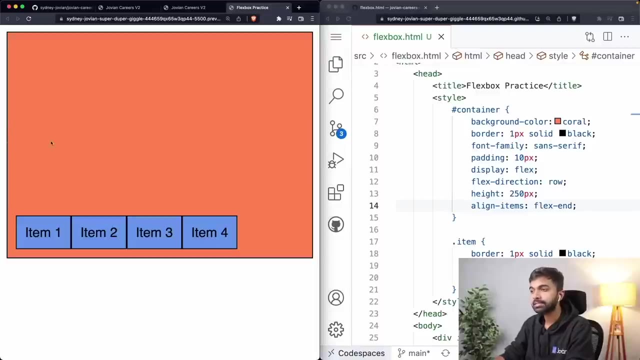 Okay, When the cross axis, this is the start and this is the end. So things are sticking to the start. Okay, I could also maybe just stick them to the end. So I can just say flex end. And now they are sticking to the bottom, which is again the main axis of the primary axis. 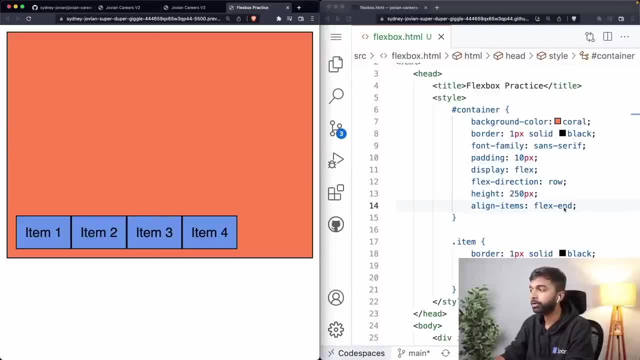 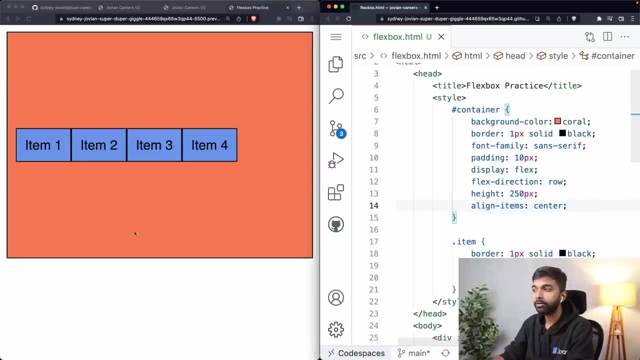 is horizontal, So along the cross axis, top to bottom. there at the bottom or at the end, I can also align item center, of course, and in which case they are centered here along the cross axis, And notice how this is different from justify content center, which is going to center them. 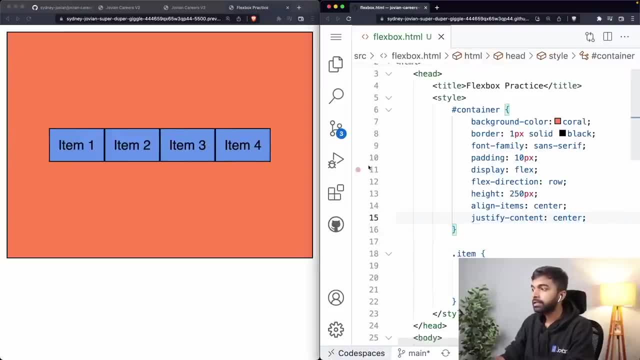 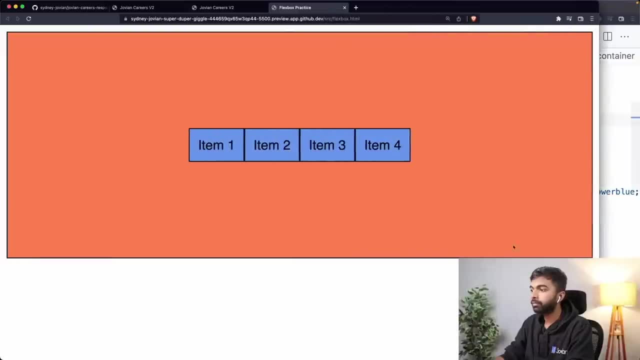 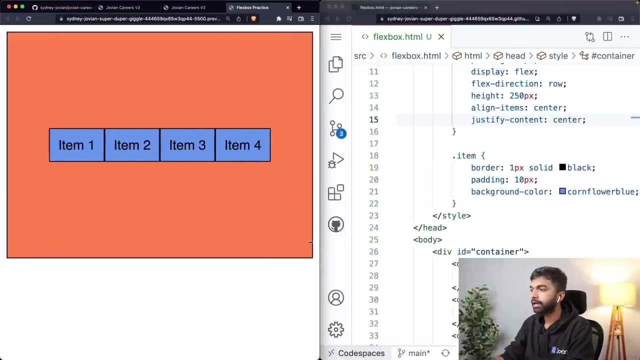 along the primary axis. So here is another trick: If you just set align item center and justify content center, then your content is centered vertically and horizontally on the page As you increase or decrease the height. it is going to be centered vertically and it. 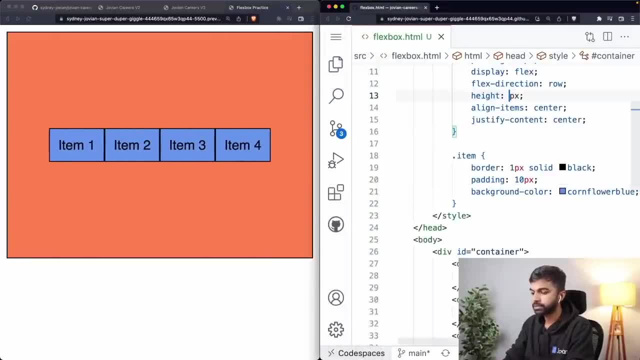 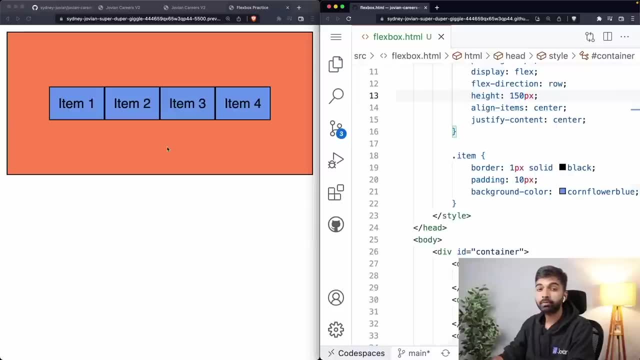 is going to be centered horizontally as well. So let's say, if this was 300 pixels, it would still be centered vertically. If this was 150 pixels, it would still be centered vertically. So vertical centering can be achieved By using the center. 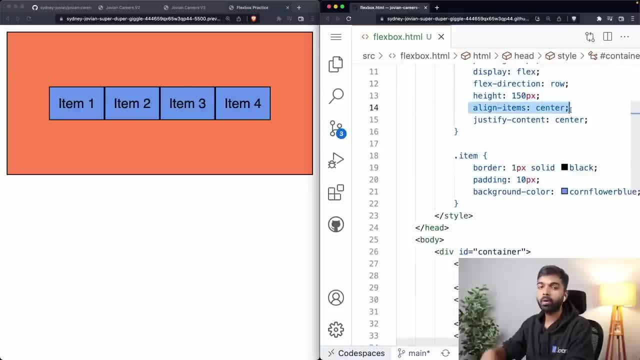 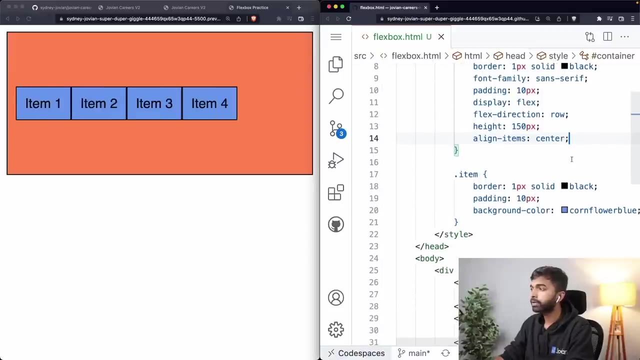 Okay, By using flex direction row, align item center or by using flex direction column and justify content center. So there are both ways to achieve it, But that is how. align items and justify content play. Justify content plays along the main axis. align items plays along the cross axis. 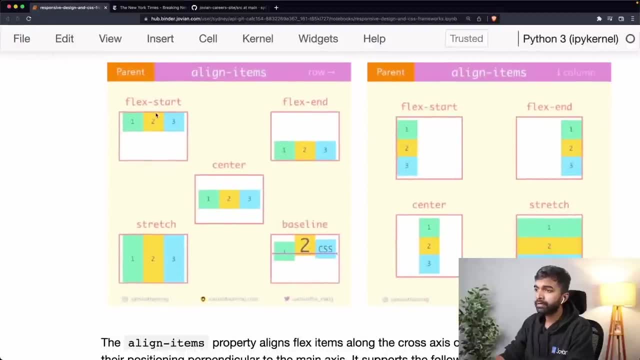 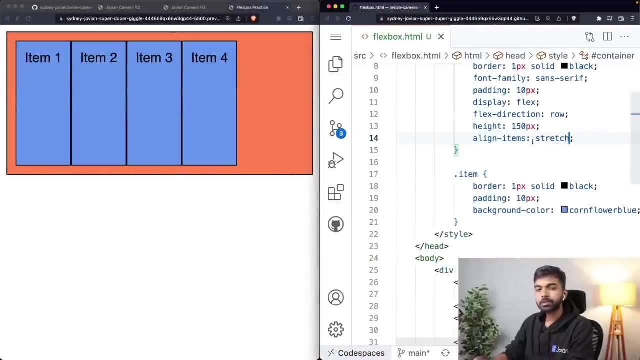 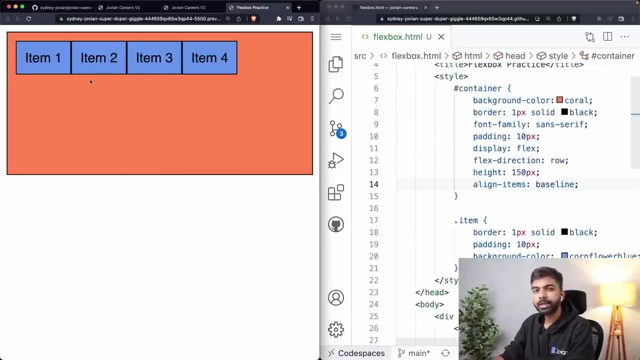 What other options do we have for align items? Well, we have flex start, flex center. We obviously we looked at stretch, which is the default value- that there is also another specific align items property called baseline, which looks quite similar to start. 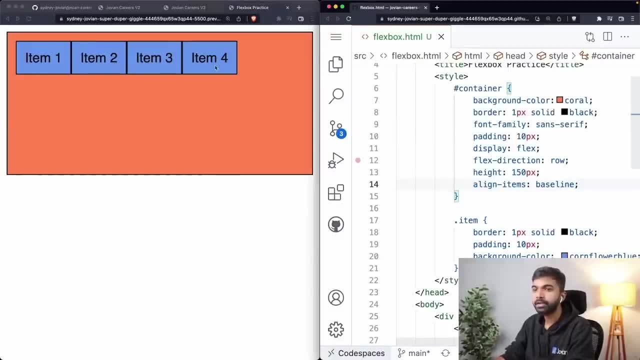 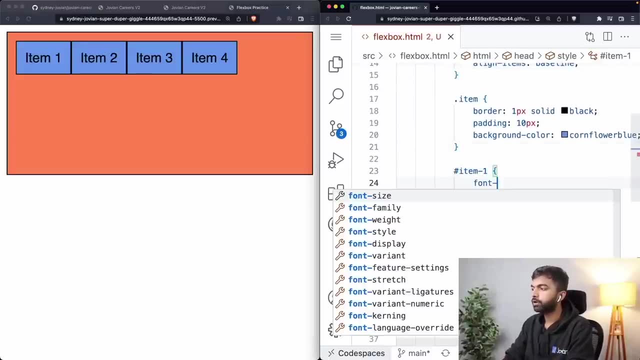 But here's the difference. What this does is this aligns the baseline of the text for each of the divs. So if I were to go in, let's say if I were to go in into item one and change the font size to 10 pixels, and if I were to go in into item three and change the font size to, 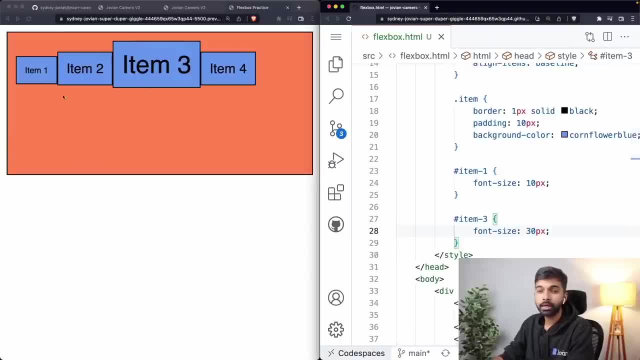 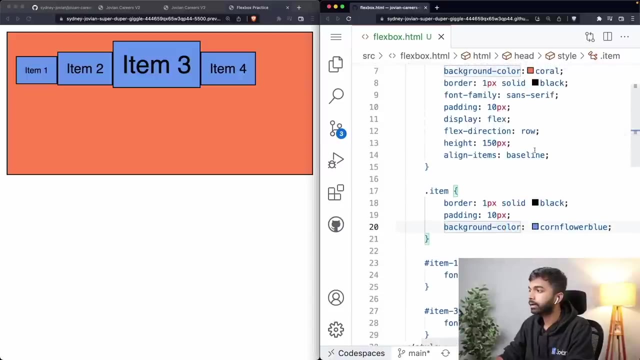 30 pixels. This is what the content would look like. So notice what's happening here. because align items is set to baseline, the line that runs through the bottom of each line of text aligns perfectly. Now, this is very different from doing align items like start, which is going to just align. 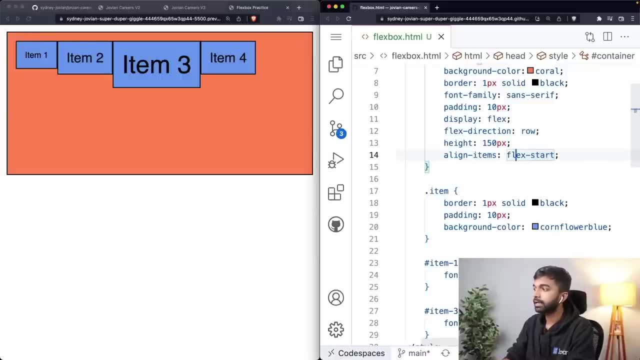 things right at the very top, or even doing something like align item center, which is going to Just say align the centers of the items and not the baseline. So the very special case- you might not always need this, but you can align by the baseline. 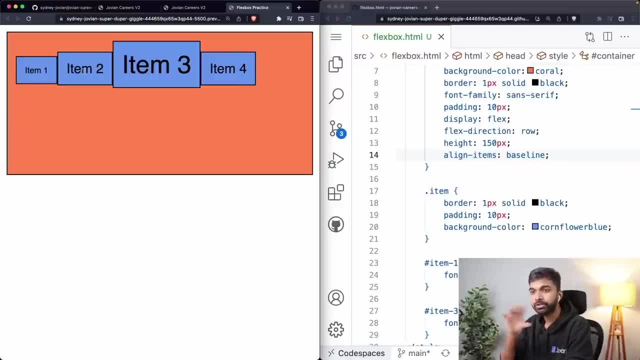 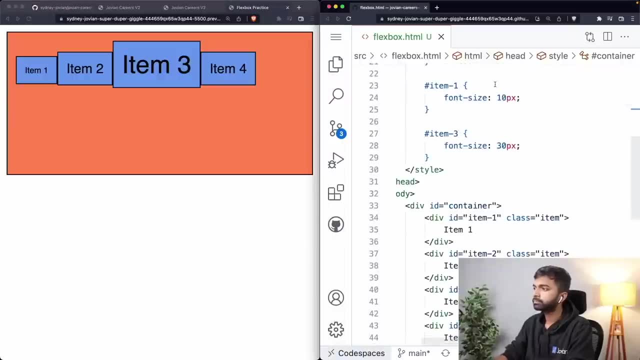 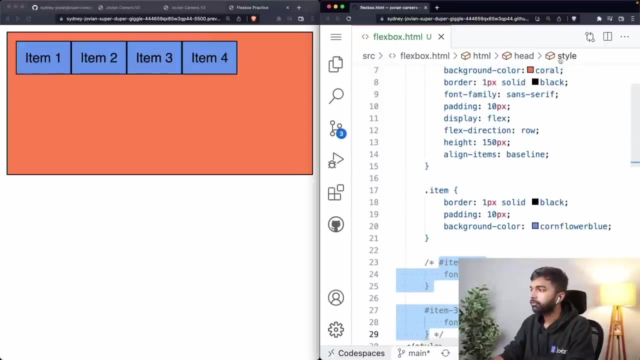 If you need to, if you have text of various sizes in a bunch of flex items. but those are all the ways in which you can use align items and let us revert that for now. And of course, all of this works on flex direction. 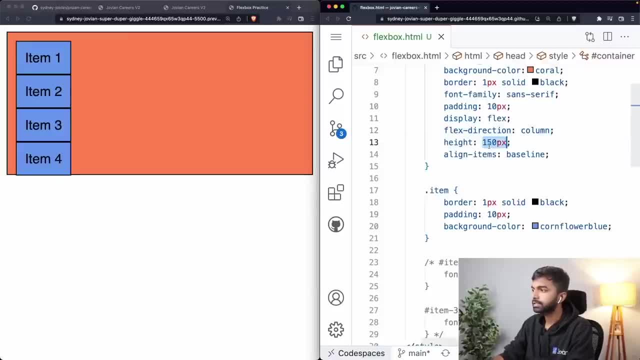 Column as well. So here we have flex direction column. let us increase this height to 250 PX. So here is flex direction column. So now the primary or the main axis is along the bottom, along top to bottom. So the cross axis is left to right. 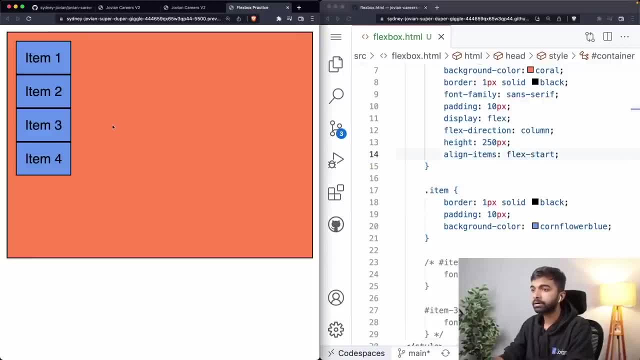 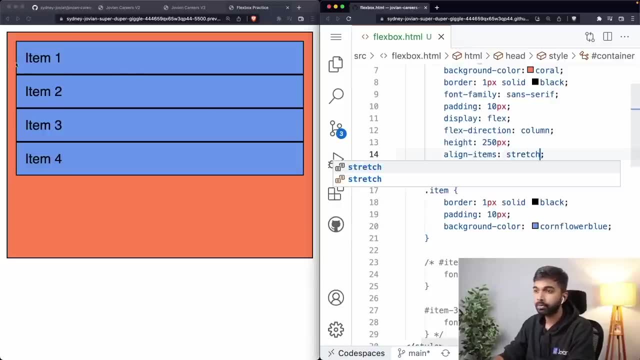 And now I could say: flex, start to align things on the left, And by default, of course, the value is stretch to align things, to take up the entire space On the cross axis, And of course I could also have align items center, in which case they will be horizontally. 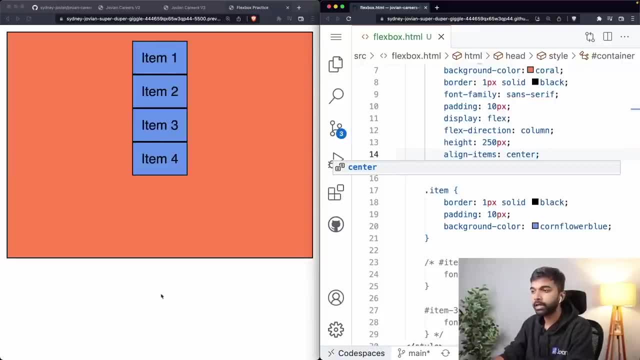 centered this time because the cross axis is the horizontal axis and vertically they're still right at the beginning. So remember that for justify content, the default value is flex start, which is right at the beginning, but for align items the default value stretch, which is to take up. 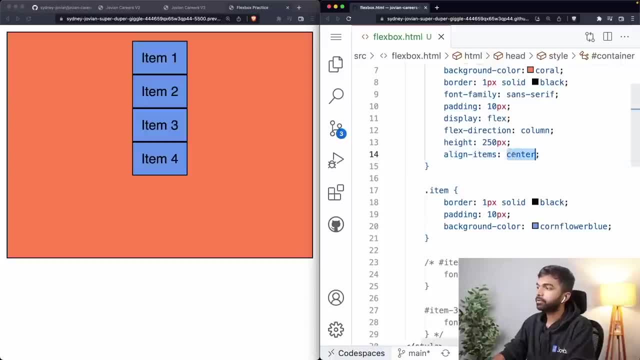 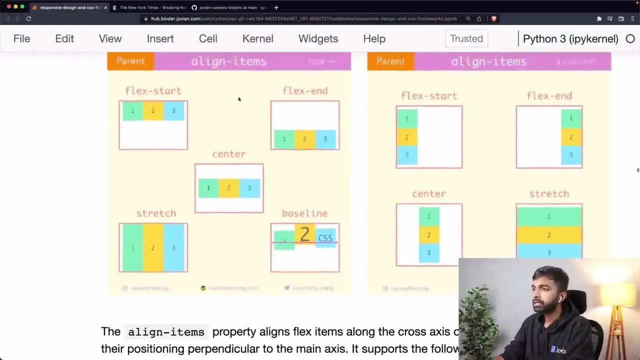 the entire space along the cross axis. Of course I can do next end here as well. Now, along the cross axis or the horizontal axis, they show up on the right. Let's reword that So: that was align items. Okay, So on. this is what it works. on row. 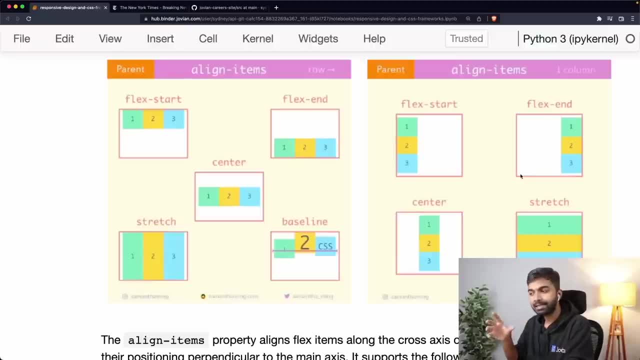 This is how it works in column. I know it's starting to get confusing. practice and that is how you will get it And, of course, you can always come back and refer to it. You don't have to remember all of this perfectly. 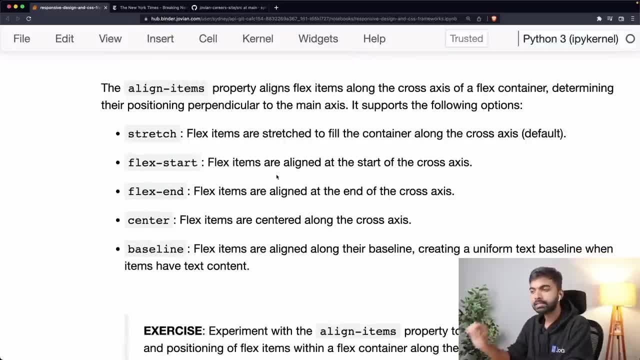 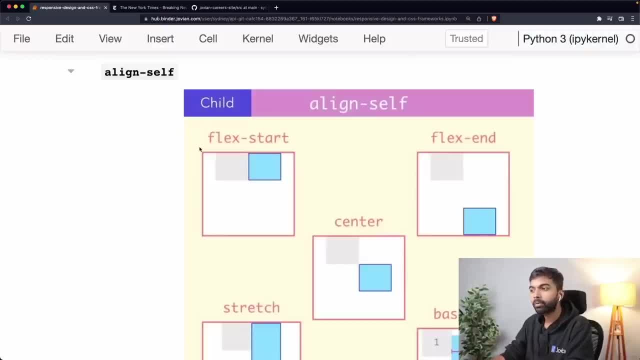 Okay, Just remember. justify content is along the main axis, line items is along the cross axis. Okay, And then you also have this special property called align self, which can be used to change the alignment of along the cross axis of just a particular child. 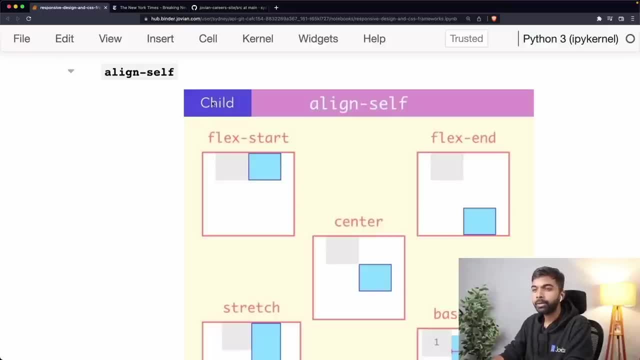 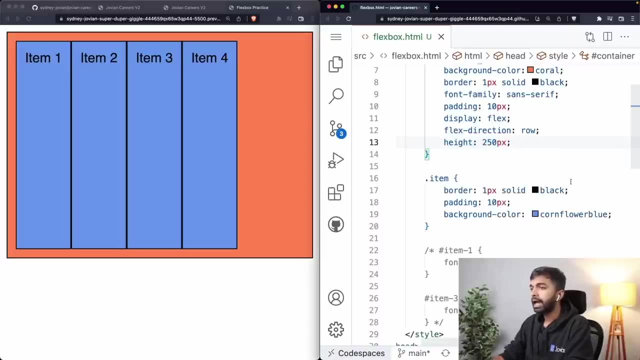 Okay, So now we're looking at certain child level properties, not the parent level properties. So let's increase the height here. Once again, I ate two 50 pixels and by default everything has aligned stretch And let me just go in here and let me just set this to align item center. for now, 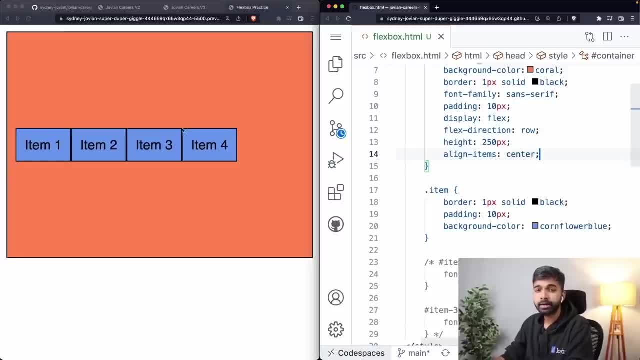 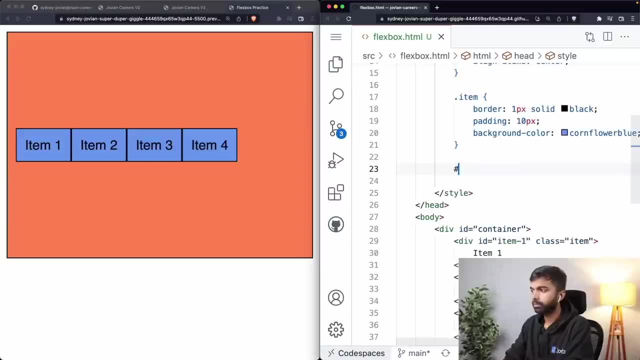 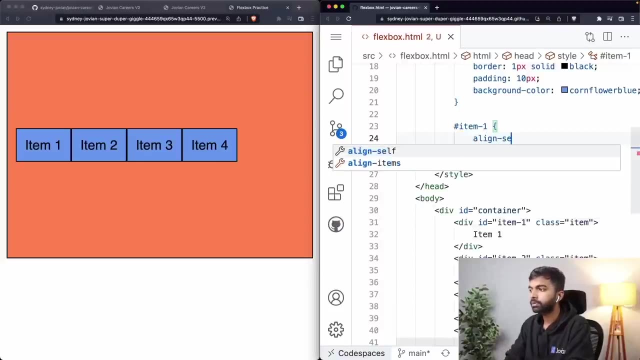 So by default all the align, all the items are aligned along the center. And let me go in here into item one, And for item one let me just set align, align self. So item one, just by itself, should be aligned to the start. 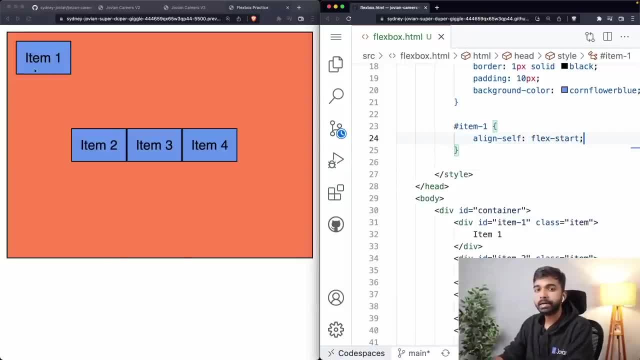 So flex start. now align items. Item one goes right, right to the top and flex start. Okay, So I can. then I can then align, maybe item to align self to flex, and I'm pushing item to right to the very end of the cross axis. 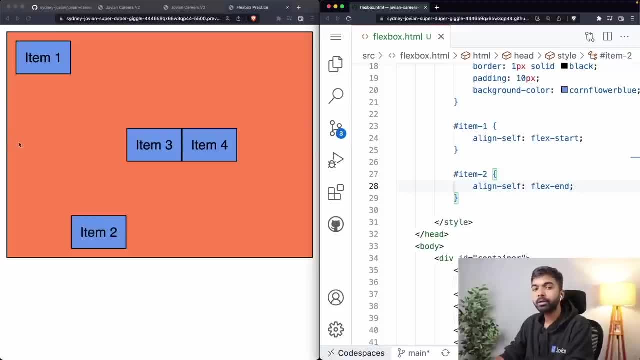 Remember, we're still on the flex direction row, So the main axis is row, The cross axis is top to bottom And we can of course go ahead. and for item three we can use line self stretch. And now item three is stretching and item four can be aligned separately as well. 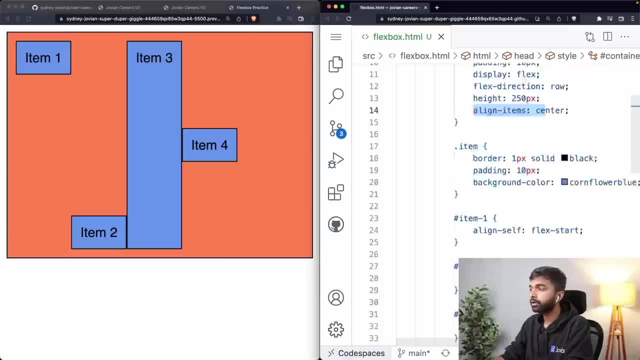 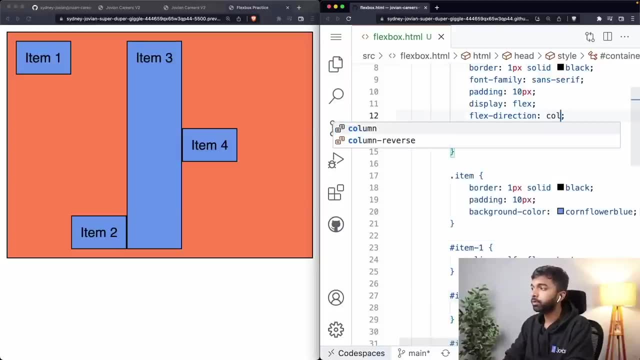 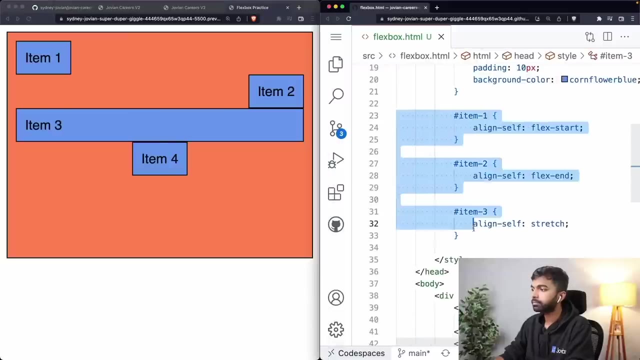 So you you can have a global setting for align items and then you can override it using align self for each item As you need. of course, this works not just for column, and not just for row, but also for column. So here now, what's happening is that we have this. let me just get rid of the default. 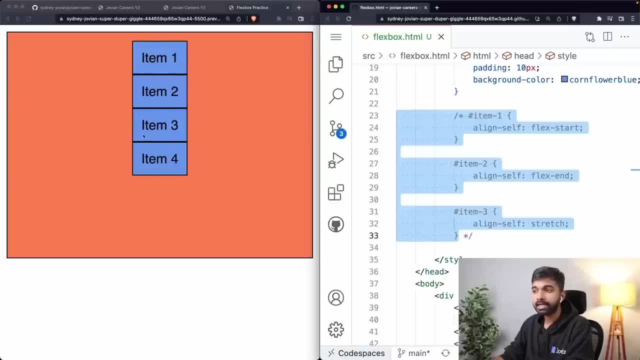 Get rid of all these for now. So now we have the column as the main axis. So along the horizontal axis We have set It to align item center. That's why they're all centered. Then if we change the setting for item one, you can see that item one goes to the left. 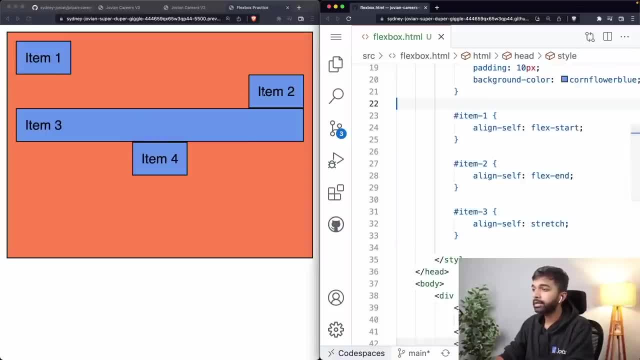 because we are setting it to flex start. Item two goes to the right because we are setting it to flex end. So, along the cross axis, which is left to right, it is going on the right. Item three is stretching and item four is in the center, which is the default setting. 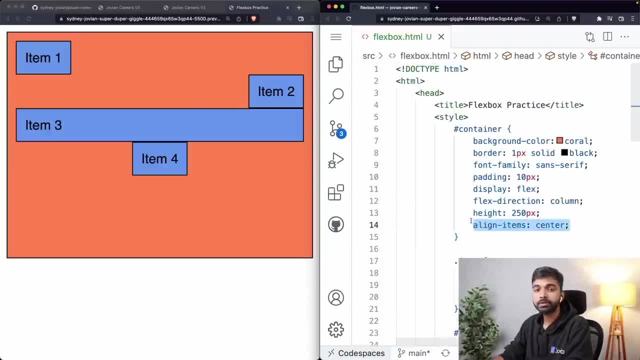 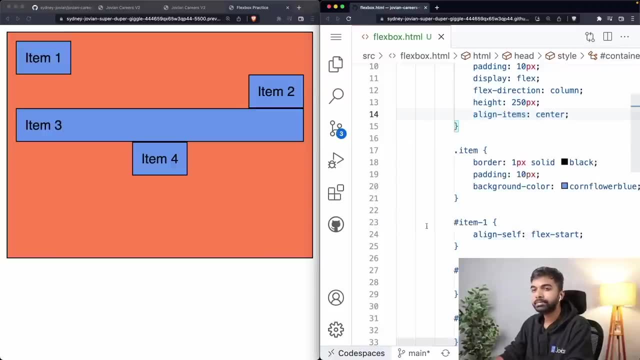 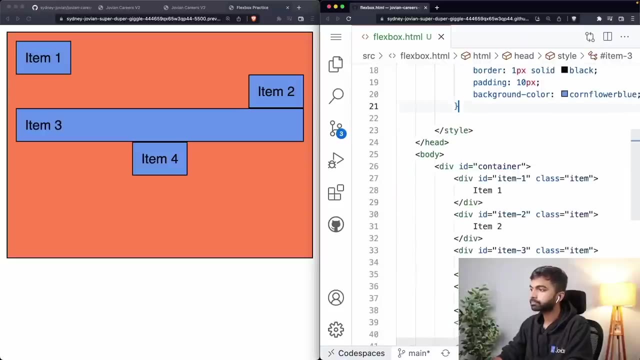 that has been put in for the container. Okay, So you can set a property for the container And then you can override it for these individual items. Now that makes sense for align items, doesn't make sense for justify content, And I'll let you think about why. for now, let's get rid of this. 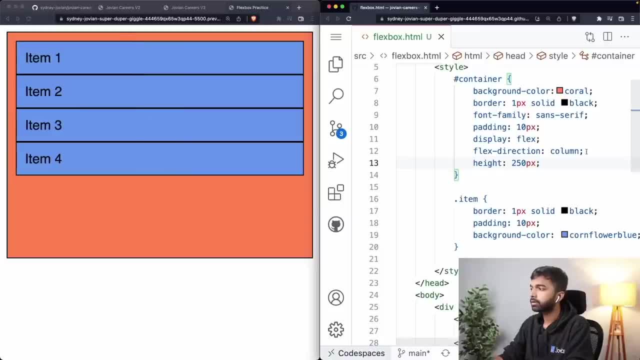 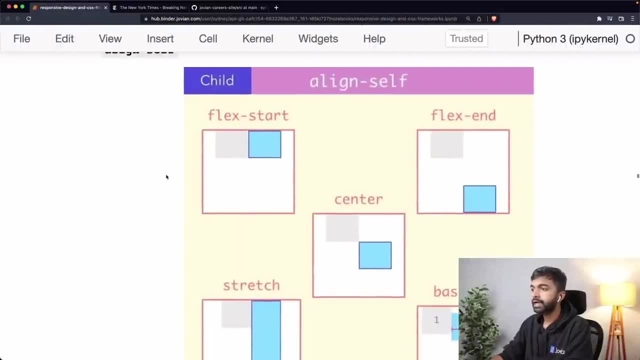 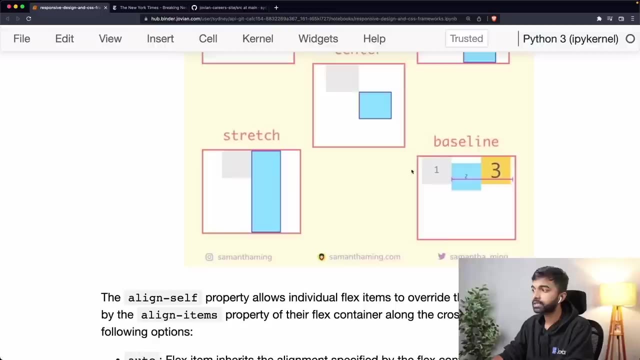 And let us just go back here to flex direction row. Okay, So that is align self. You can use flex start or you can use flex end to move it to the end of the cross axis. You can center it in the cross axis or even stretch it, or even align it to the baseline. 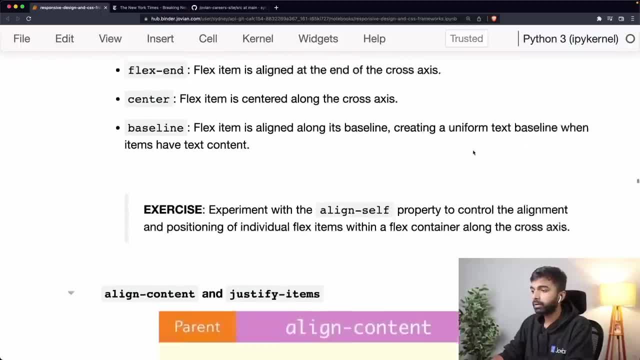 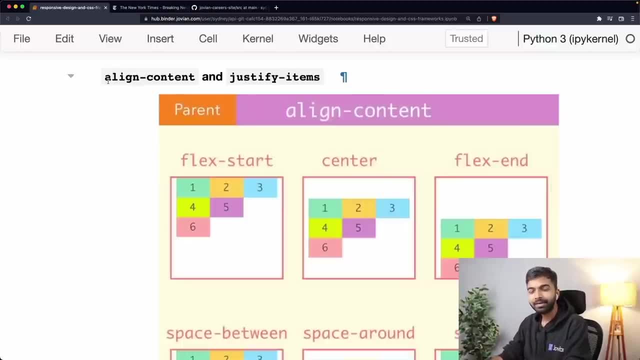 You have all these options available to you, Okay. Next up, there are also a couple of adjacent properties called align content and justify items. I will not cover them here because they are not very commonly used. I have almost never used them, maybe once or twice, but they are slightly different from. 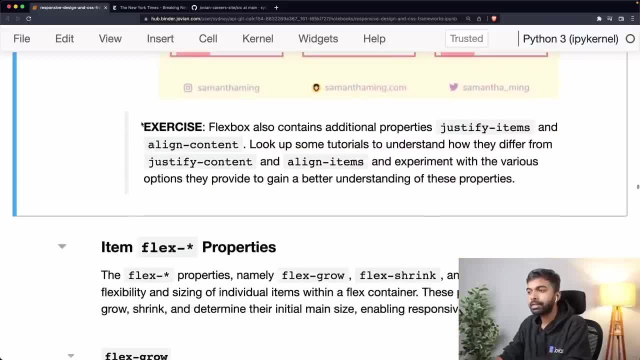 align items and justify, justify content. So I will let you explore these on your own. So check out the properties, justify items and align content As you can imagine they might do. alignment along the main axis and justification along the cross axis, So you have those options as well. 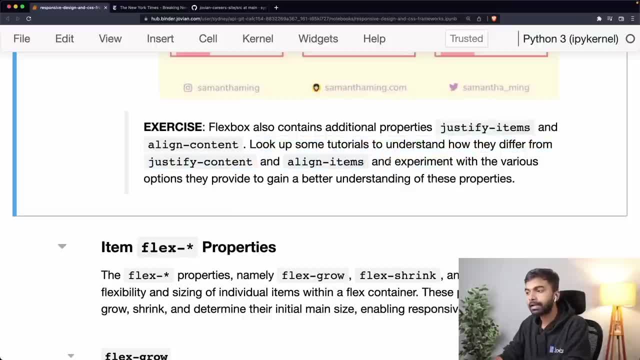 And look up some tutorials to understand how they differ from justify content and align items. Or, if you don't want to get confused right now, just skip these all together and just use the default justify content along the main axis and align items along the cross. 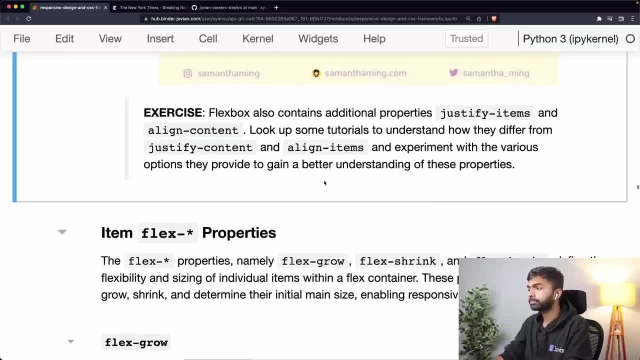 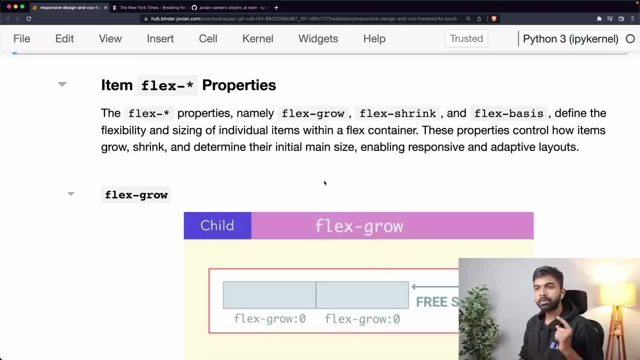 axis. But if you want to, you can experiment. Okay, So those are some justification and alignment properties. So in most cases, you will be working with flex direction, you will be working with flex wrap, you'll be working with the align items and justify content properties. 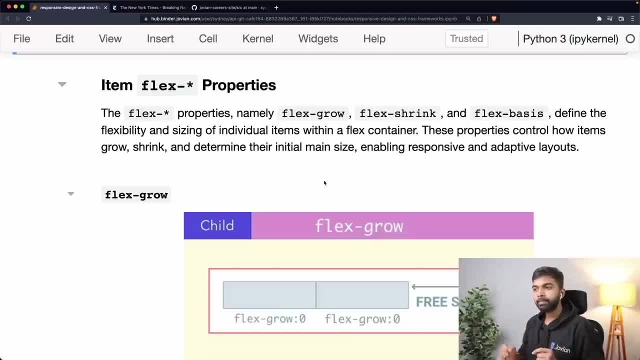 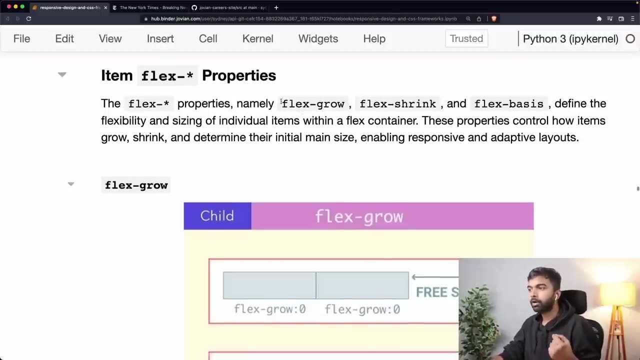 And sometimes you will use the align self property on a particular child. But then there are also certain flex properties that you can set on children specifically to control How the various children take up space on the page. Okay, And we're going to look at all of these properties. they're called flex grow, flex shrink and 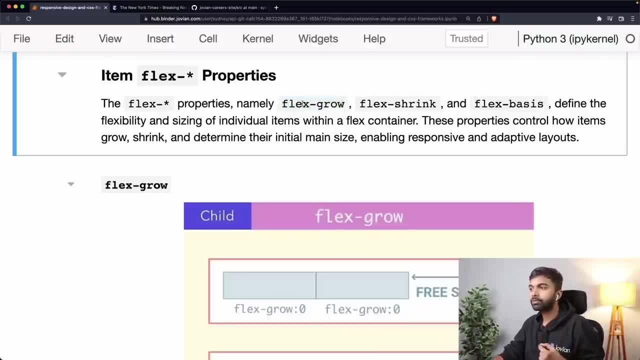 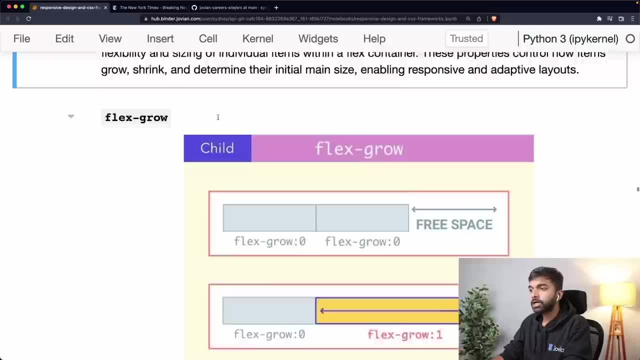 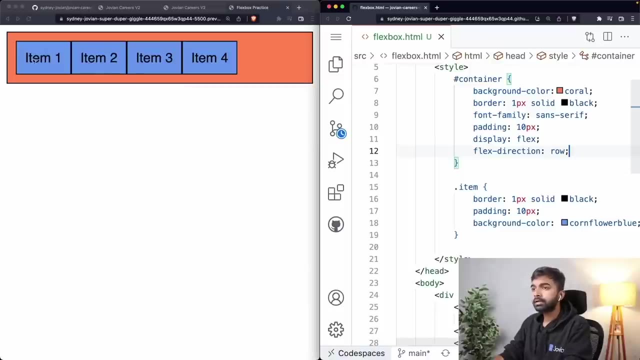 flex basis And then we're going to look at a shorthand property so that you never actually have to use all of these separate properties. but it's useful to understand what they mean. Okay, So the first property is the flex grow property. Now notice over here, if I get rid of the height notice- that these tips are not taking. 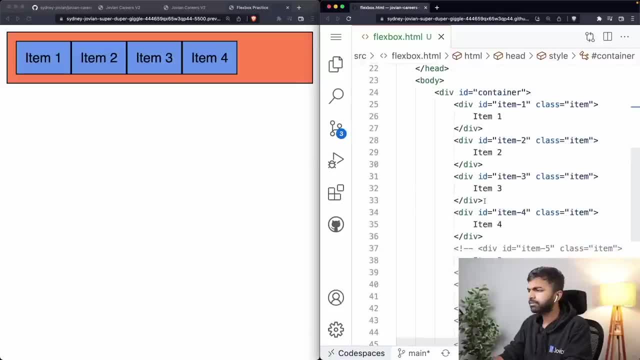 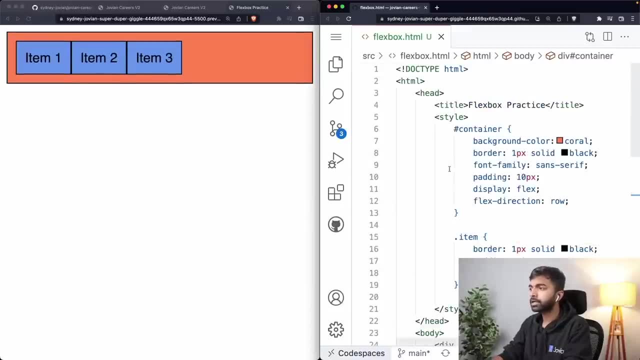 up the entire space And these. then let me just have three dips for now. let's get rid of. get rid of the fourth div as well. Yeah, so notice that these dibs are not taking up the entire width on the page. Now, sometimes you might want in maybe some kind of a sidebar layout where you have a 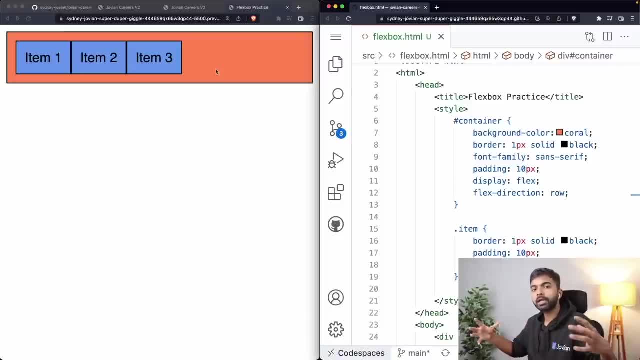 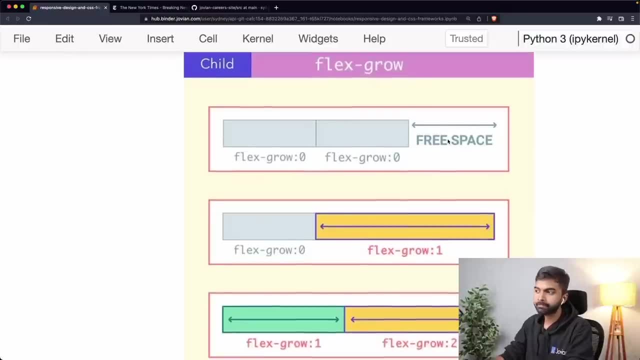 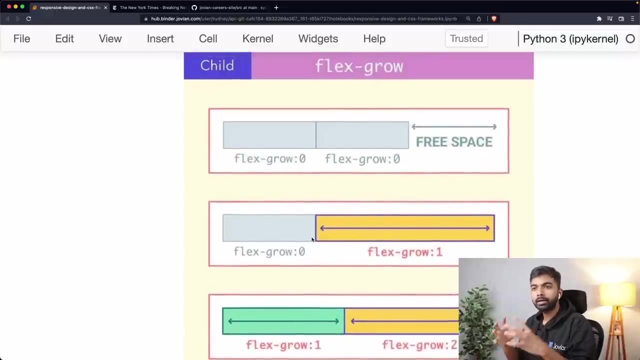 left sidebar, right sidebar and the middle item should grow to take up as much space as possible. In such cases, you can use the flex grow property. So when you have some free space, you can specify a flex grow property and by default its value is set to zero, which means that you don't want a and you don't want one of. 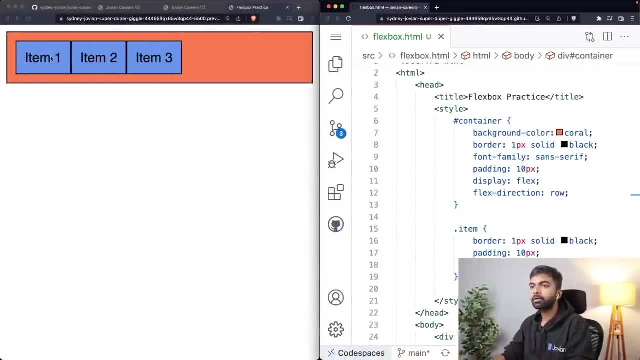 the children to grow. by default, you only want each of the children to take up as much space as is required to display all of its children. Okay, so for example, right now to show item one, this is the only amount of space that. 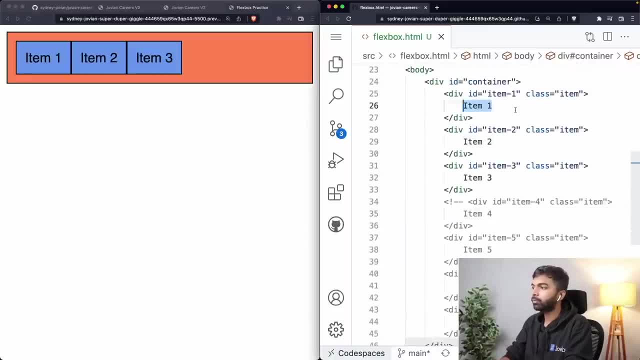 is required. But if let's say the text here was item one, item one it would go. it would take up twice the space to show the, to show the content right. However, if let's say I wanted item two to take up all the space in between an item three, 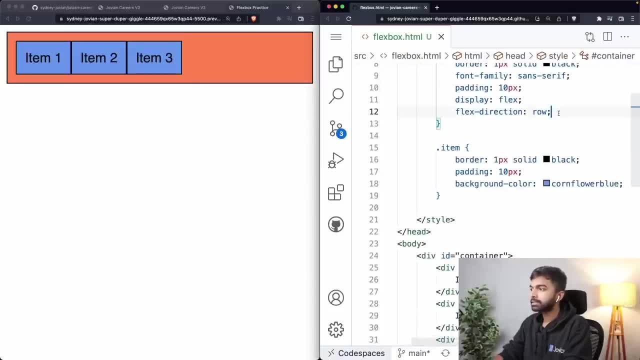 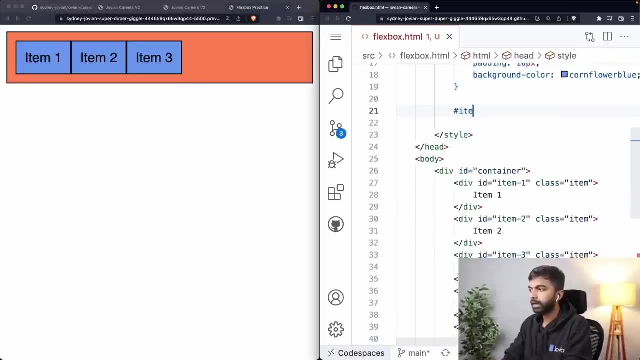 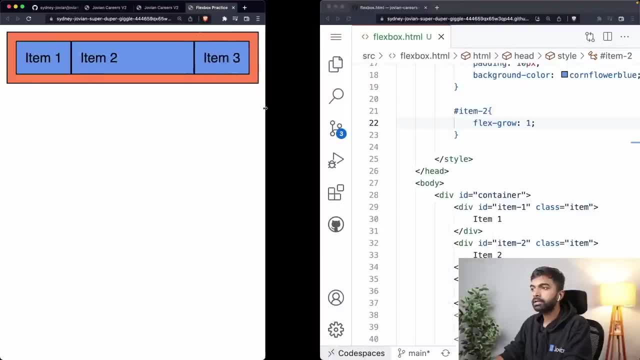 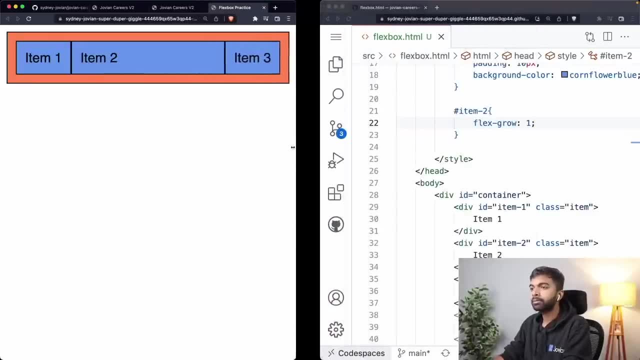 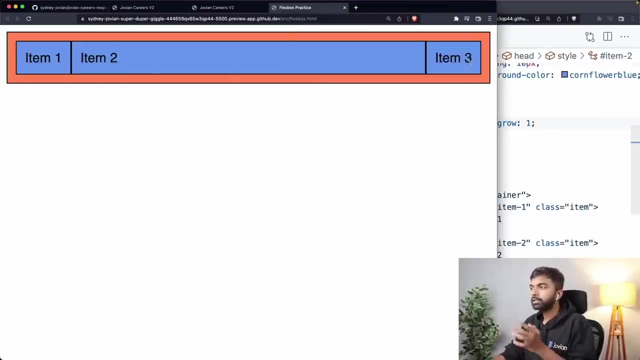 But as soon as, as soon as you specify something other than zero, item two starts to grow, to take up the available space. Now let's say I wanted to do something slightly more complex. Let's say what I wanted to do was item one should take up maybe 30% of the space. 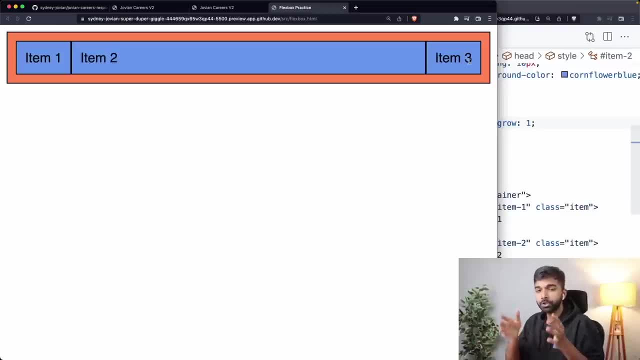 Item three should take up 30% of the space and item four should- item two should take up 40% of the space. there should always be. if there is additional space available, it should go 3040- 30.. Okay, let's do. let's see how to do that. 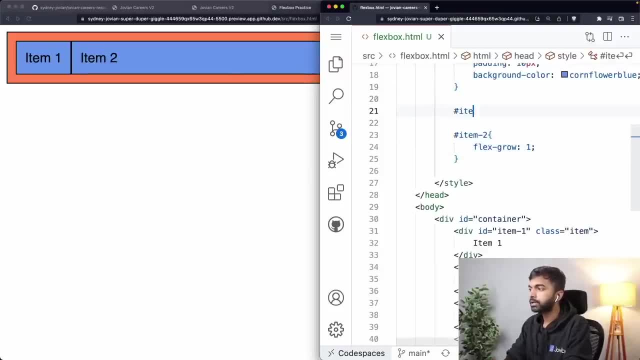 So the way I would do that is simply by specifying those proportions for each item. So for item one, let us say, flex grow to be three, And these are proportions. So that's why I don't necessarily need to write 3040, 30, these are not percentages. 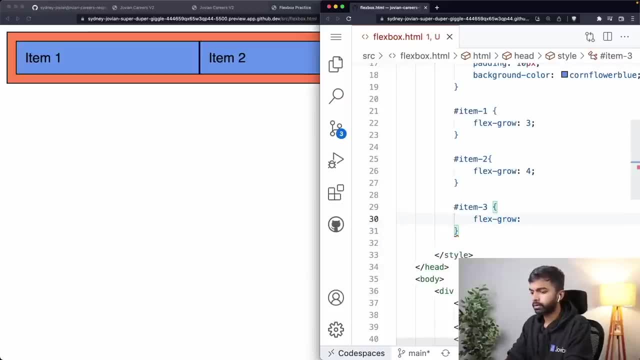 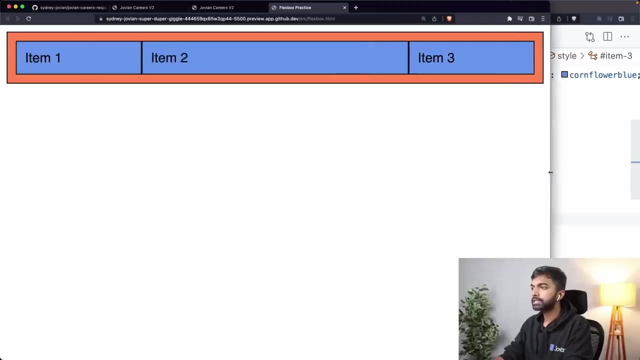 And item three will also be flex grow. Now you can see this layout 343.. And maybe, just to make it a little more pronounced, you can look at maybe 262.. You can see that 20% of the space is taken up by item. 20% of the space is taken out by 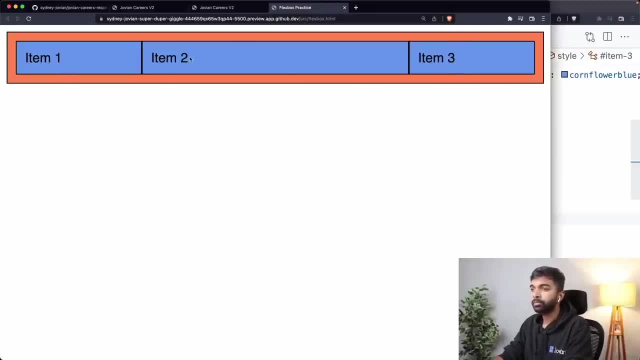 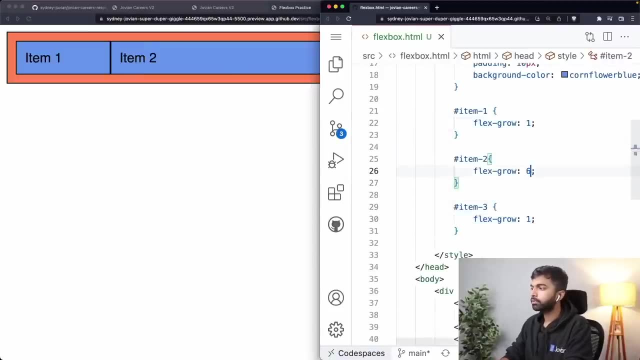 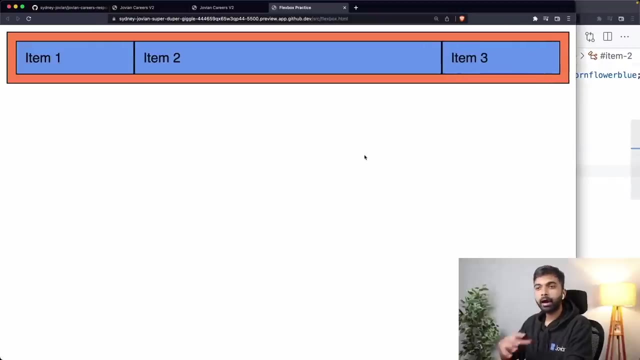 item 120% by item three And you can see that item two takes up about 60%. Okay, you can also do something like 11 or they don't have to add up to 10 or 100 or anything. It's just that now you can see that out of the additional space that is available, 10%. 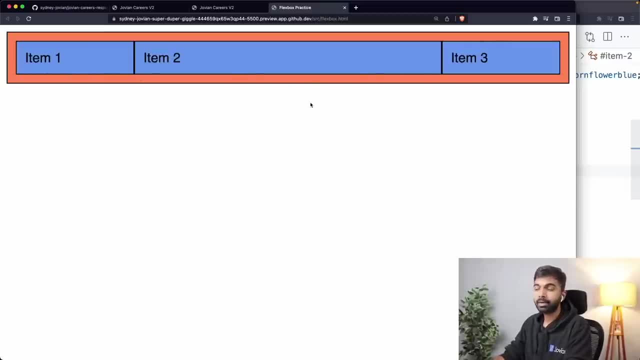 of the space is taken by item 110% by item three and the rest is taken by item two. So what you're specifying is, among the available additional space, how much space should be taken up by each item? how much additional space? so these are not exactly in that proportion. 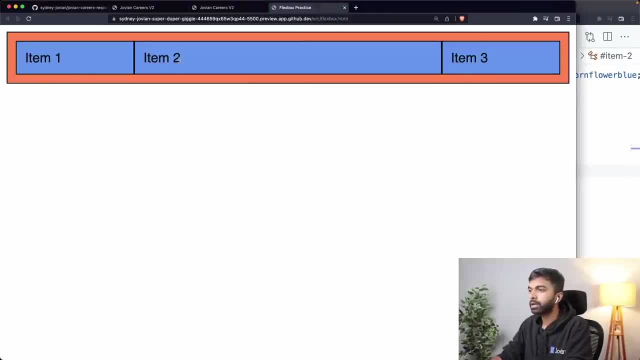 These are actually not exactly. one is to four is to one, Okay. Okay, Because the base size is not affected. That is where we talk about flex basis slightly down the line. But grow tells flex. grow determines a flex items ability to grow relative to other items. 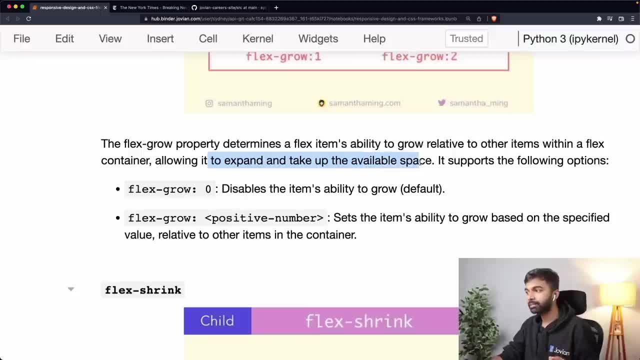 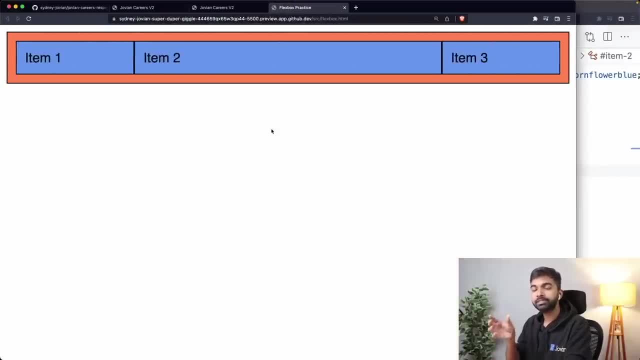 within a flex container allowing it to expand and take up the available space. So what you can do is you can say that, out of all the additional space, how should that space be distributed to each item? and the? by default, it is zero. 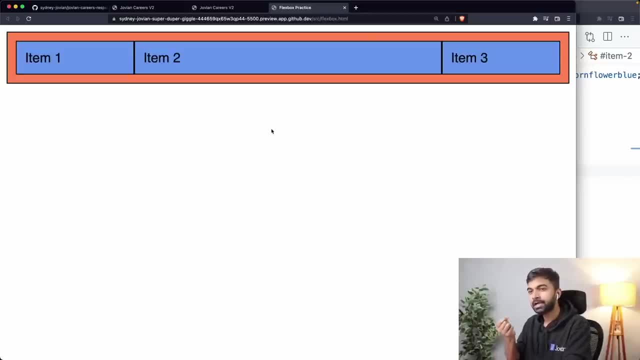 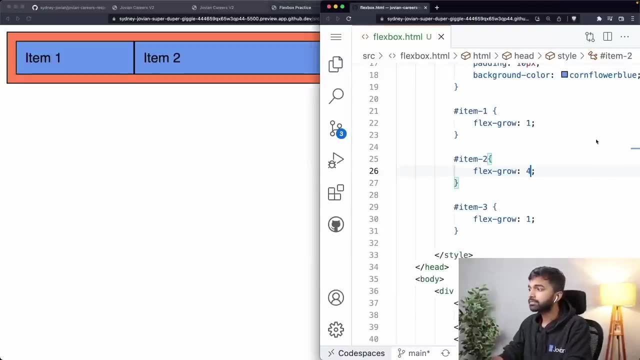 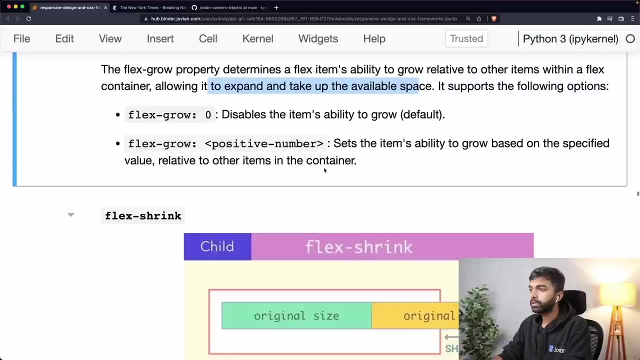 So by default, the additional space does not go to any item, And as you start setting values for each item, then don't buy those proportions. the spaces distributed: Okay. So that is flex. grow Next up we have something called flex rank. 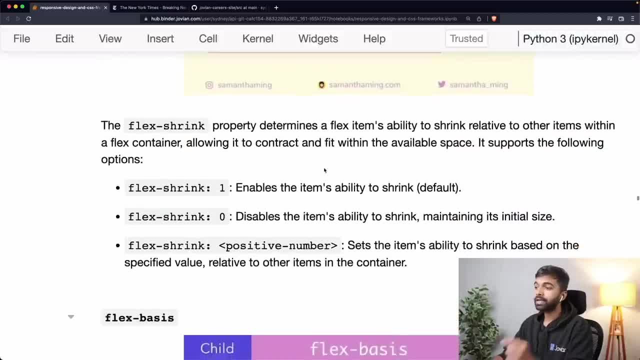 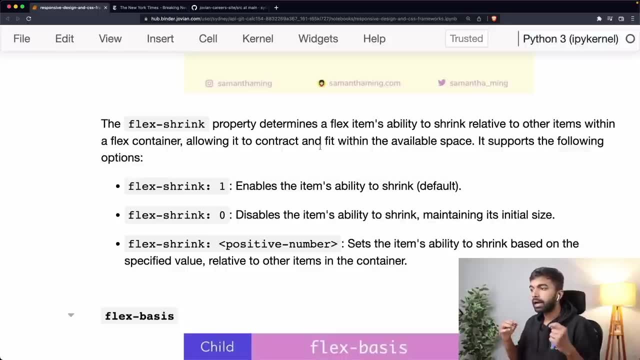 Now, just as we have flex grow, we have the flex shrink property, and the flex shrink property determines a flex items ability to shrink relative to other items within the flex container, allowing it to contract and fit the available space. So here is how it works. 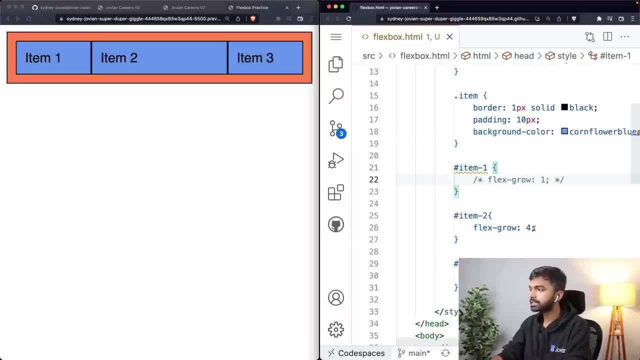 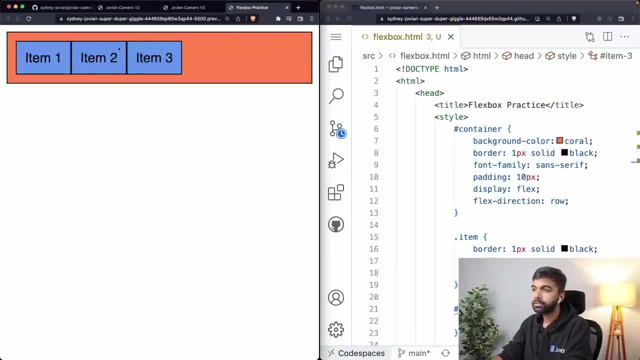 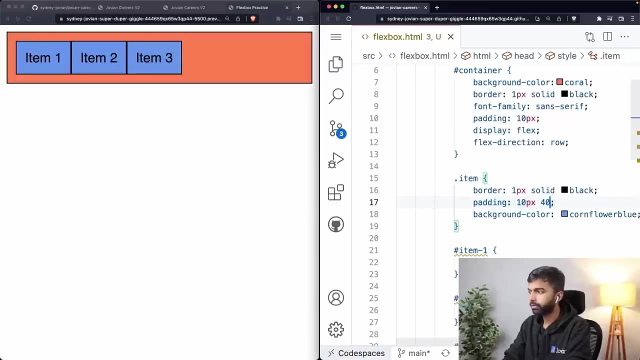 Let me get rid of flex grow settings for now. Let's just disable this, disable this, this. So now let's say we had too much content here and we had to actually shrink things. How can I do that? Well, let me just add a bunch of space here. 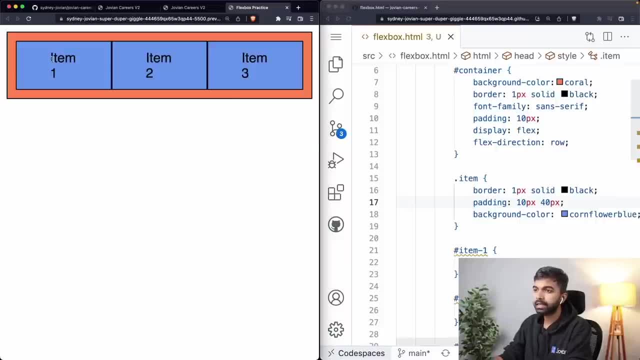 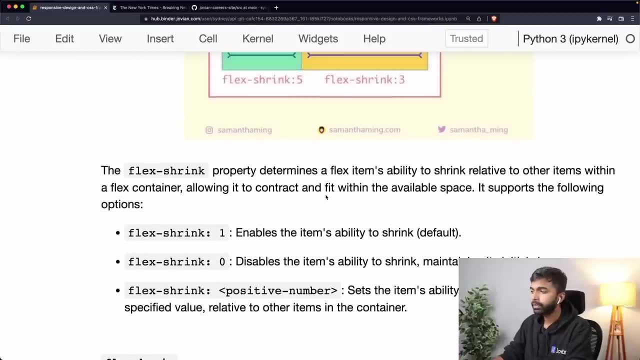 Okay, so now there is. now there is more space here And you can see that the text is wrapping onto the next line. But if we wanted to, If you wanted to shrink things a little bit, then we would have to go in and set the shrink. 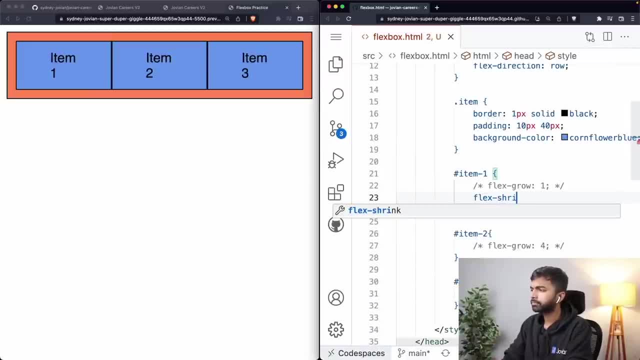 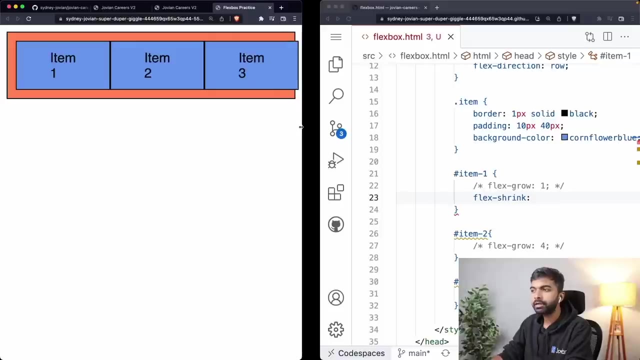 property. Let me set your flex shrink And by default things shrink automatically. So this is the default value. So you can see that they have shrunk a little bit. Ideally they should have been like this, But they have shrunk a little bit. they have shrunk a little bit because the text has come. 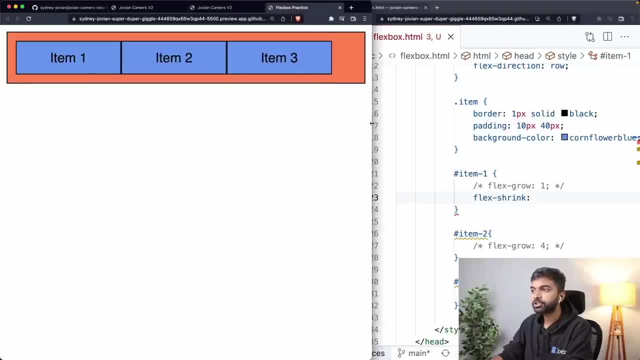 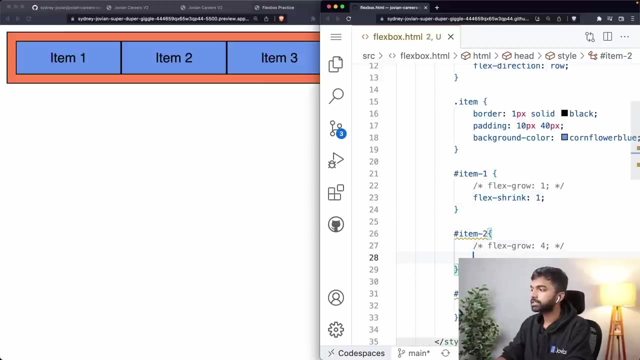 onto the next line. So there's definitely some shrinking that has happened. So shrinking is happening by default and they're going to shrink to their base size and they're not going to shrink beyond the base size by default. But in case I set flex shrink to one or one of them and then I set flex shrink to zero, 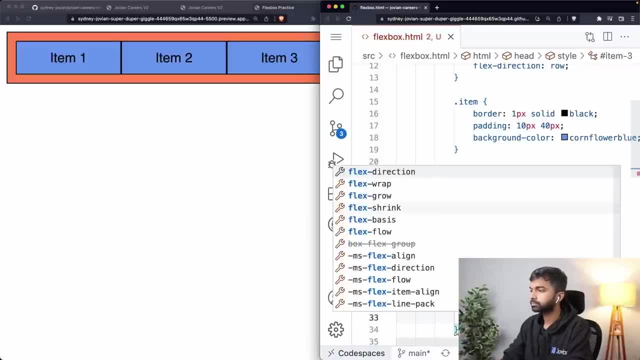 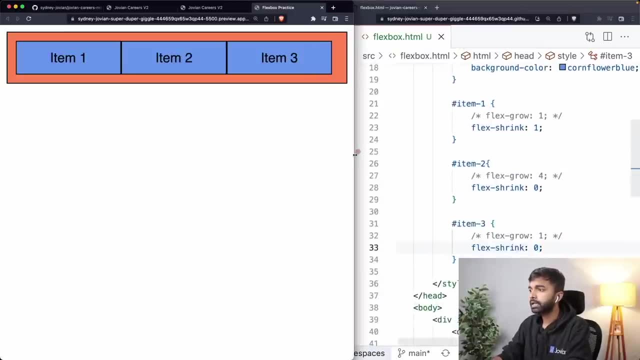 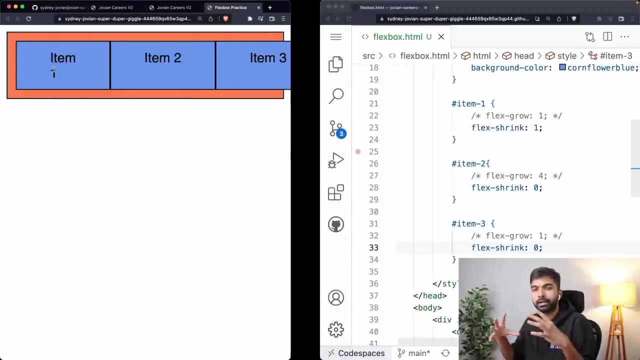 or the others. So I've set flex shrink to one and flex shrink to zero. Okay, Flex shrink to zero. You can now see that as I shrink it, item one shrinks, which is a default. it tries to shrink So till it can no longer shrink, till there is no, till the space of its children is completely. 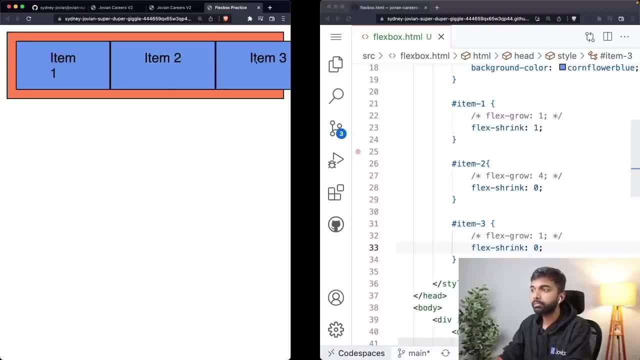 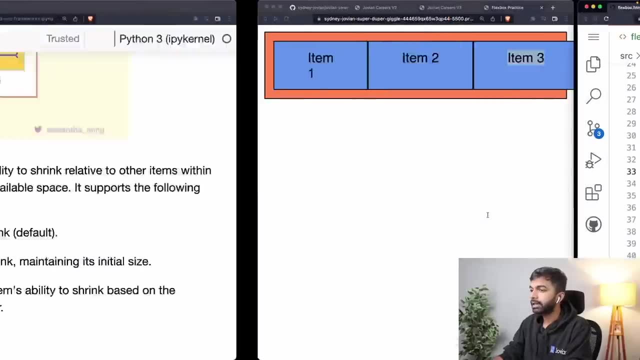 taken up, But item two and item three don't shrink, because the shrinking is constant. That's what happens, And of course you can then shrink in proportions as well. Let's say, you set it up in such a way that Each of these are taking up some additional space. 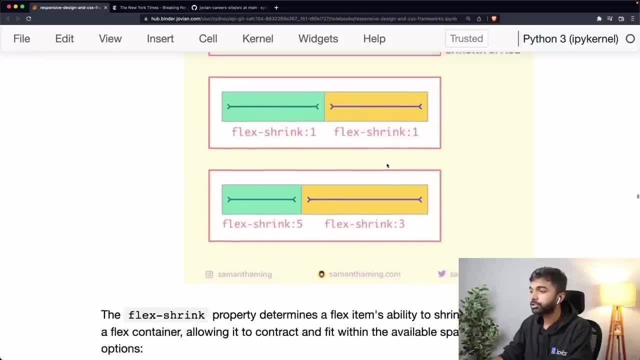 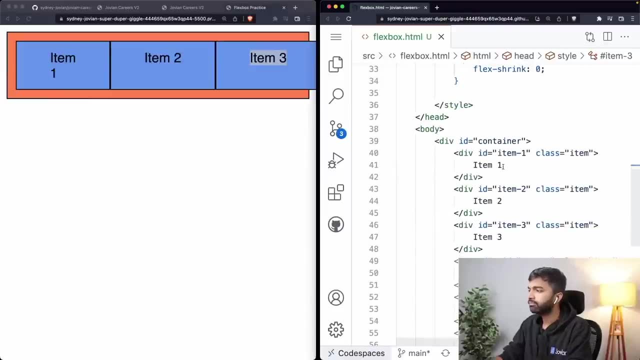 You have original size, original size here, and you're then going to try to shrink them in a certain proportion. So item one is going to shrink in a certain proportion. Item three is going to shrink in a certain proportion. This will be clearer if we have more content here. 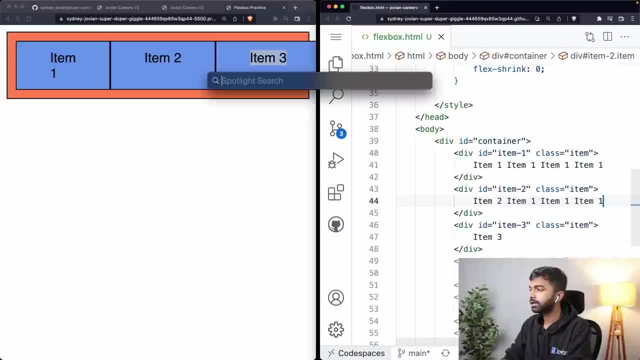 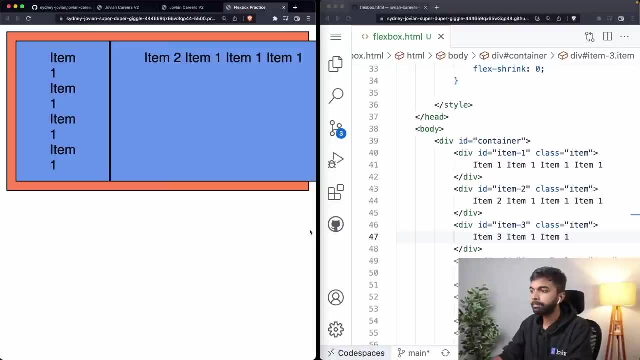 Let me just put some more content so that each of these can shrink independently. Okay, Now you can see that item one has shrunk significantly, whereas item two and item three have not shrunk at all. But let's say, we want the shrinkage to happen in a certain proportion. 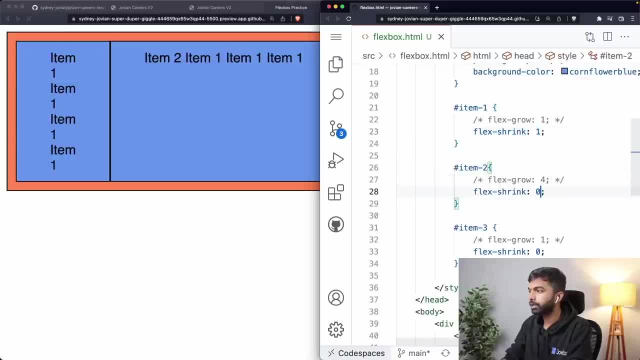 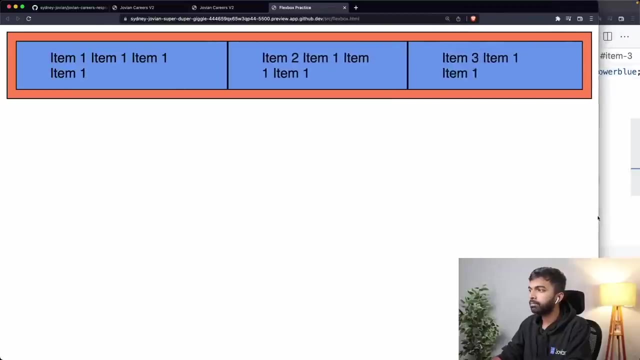 So then we could say that, okay, item one should shrink in the proportion of one item, or two should shrink in the proportion of three, So it should sink three, X, and item three should also shrink proportion one. right, You can now see that right now item two is shrinking the most, whereas item one and item 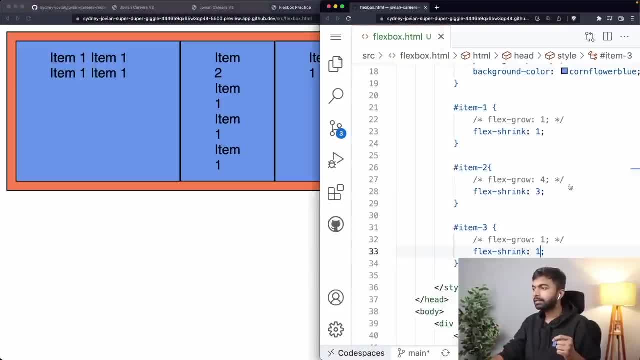 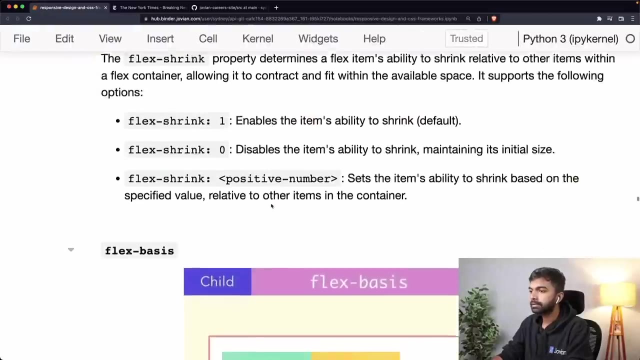 three are shrinking the least. So what we are saying here is that The Flex size has to be distributed in the ratio one is to three is to one for the specific columns. Okay, So that is flex shrink, And then the final, the final property is flex basis. 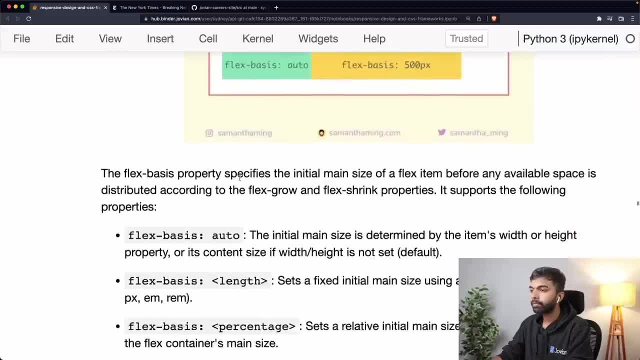 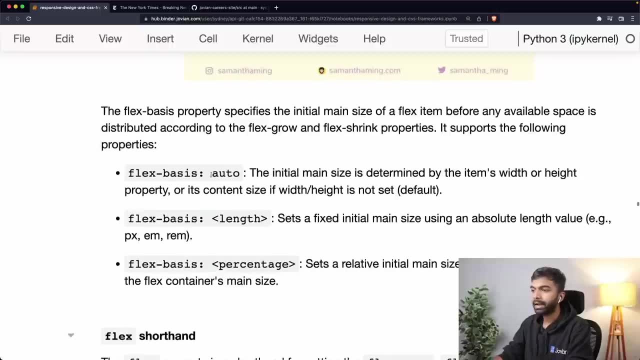 Now the flex basis property decides what is the initial main size of a flex item before any available space is distributed, And by default, the flex basis is set to auto, Which means that The main size of each child is determined by the items own width and height, which is 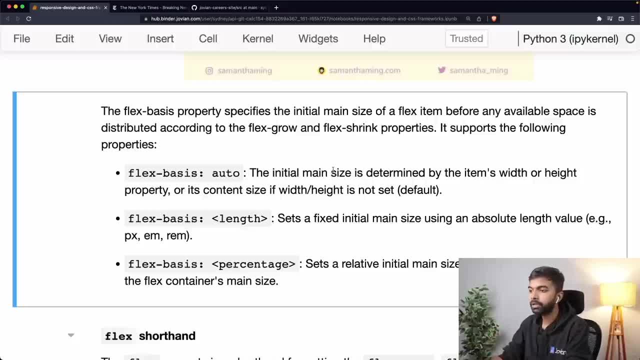 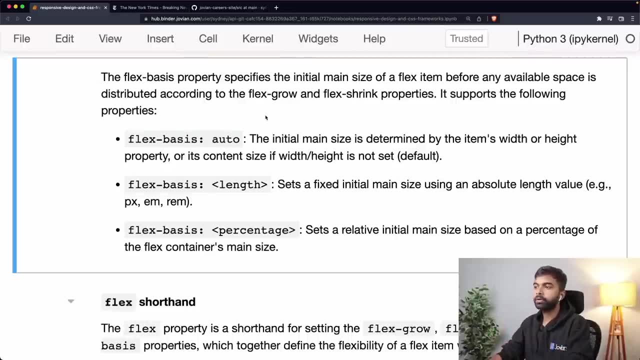 basically the width and height of its content. If it is not set Okay, However, you can also say that the basis or the main size of our of a particular item is zero, So let's see what happens when we do that. 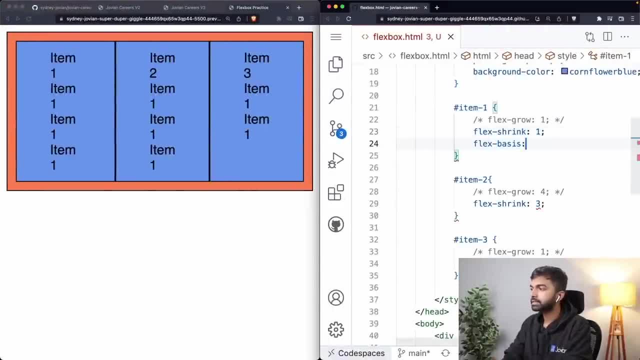 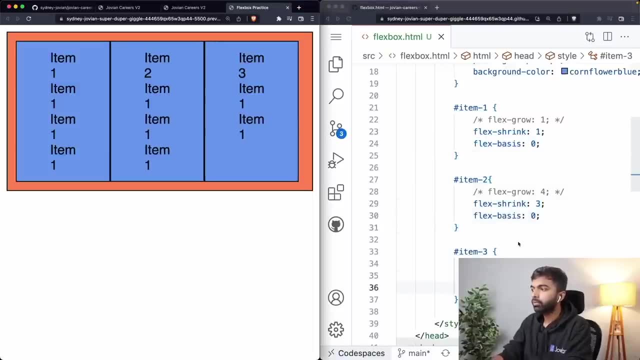 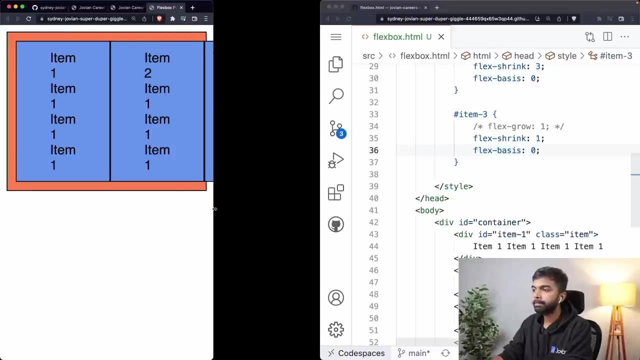 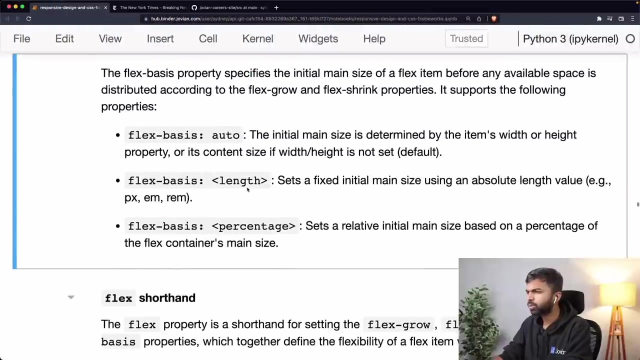 Let us set flex basis to zero for all of these. Okay, Now, when we set the flex basis to zero, what we're saying Is that there is no basic size. You can keep reducing the size, and I think I guess it's one probably. 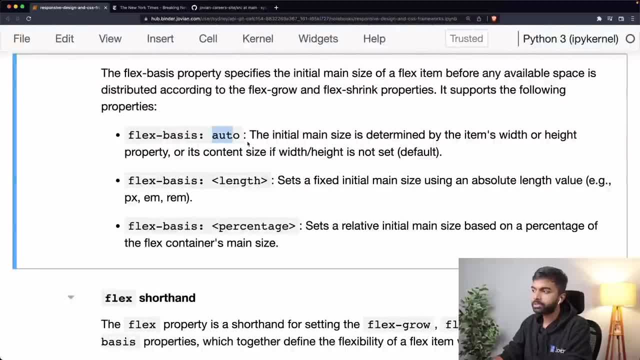 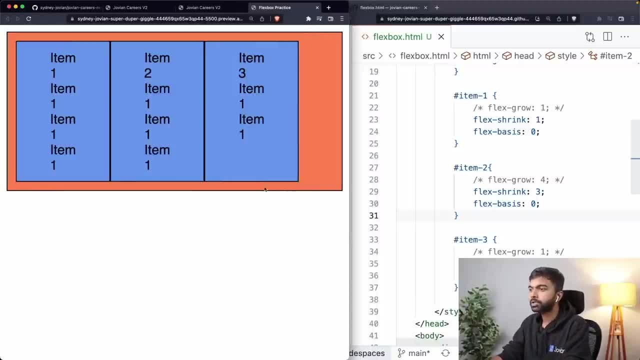 Yeah, So by default flex basis is set to auto, which means it takes up its default size and then flex basis of zero says that there is no basis size and it can shrink as much as possible. So in this case you can see that item one, two, three are all shrinking as much as possible. 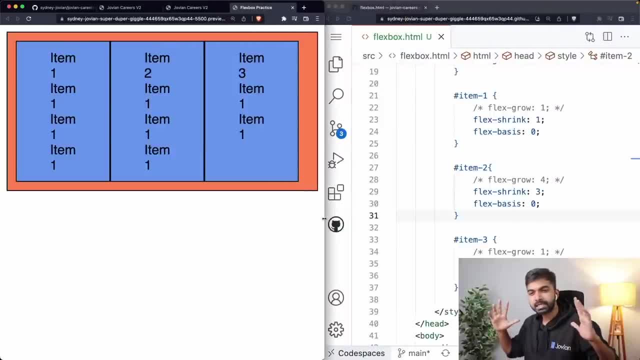 Because we've not set a basis size, So the basis size is just as low as possible, right? So by default there's no shrink. There is no, it is not going to take up any additional space than the minimum necessary space. 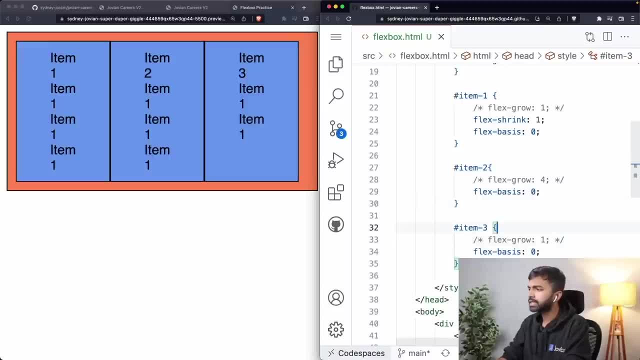 On the other hand, and when flex basis is zero, strength doesn't really make sense. On the other hand, we can add flex grow, And now what we're saying is that they can grow to take up the additional space In the specified criteria. 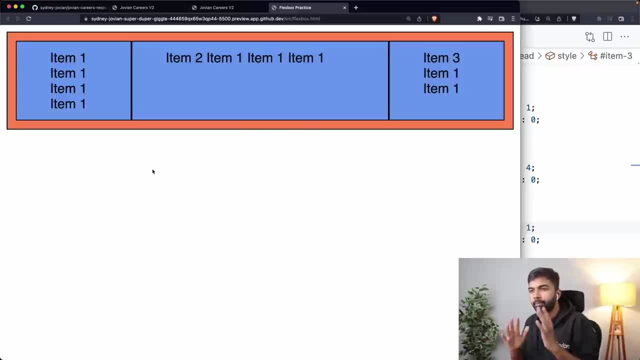 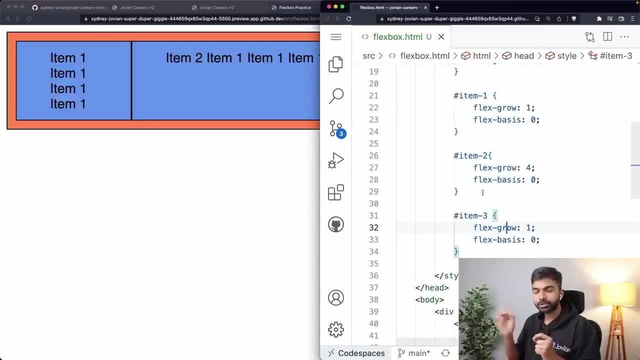 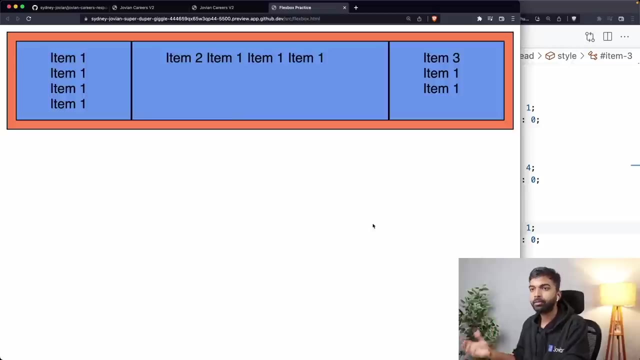 So one is two, four is two, four to take up whatever additional space is available beyond the very basic minimum base. Okay, So the interplay of flex basis, flex rank and flex grow is what decides what happens in the default state, What happens when you have more space available. 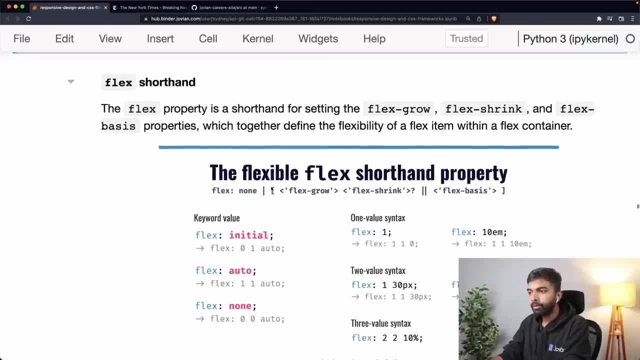 What happens when you have less space available? Okay, But, however, most of the time you don't actually use these three properties. You just use a basic value, Okay, So you just use a simple shorthand property called flex, Okay. So here's what you can do. 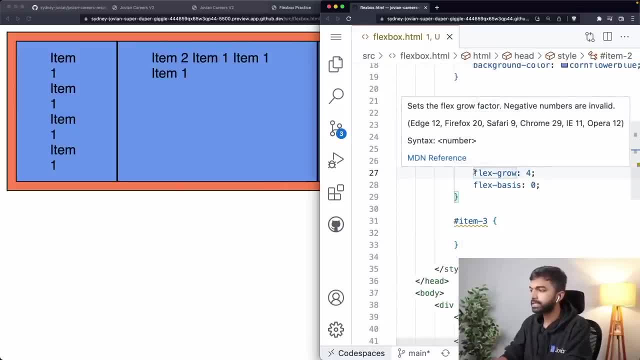 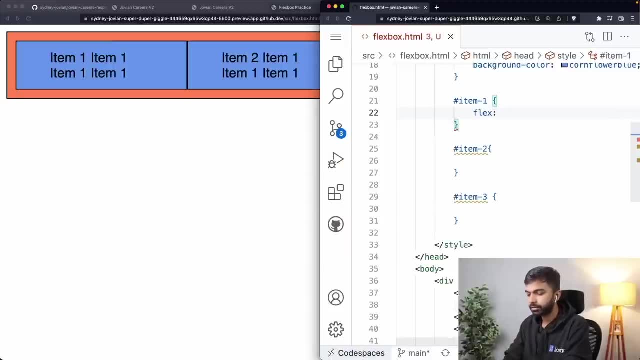 Instead of saying flex, instead of saying flex, grow, flex, basis, flex um rank, et cetera. Let's say, I want the ratios to be two, four and four, at least the ratio of the additional space and the shrinkage. 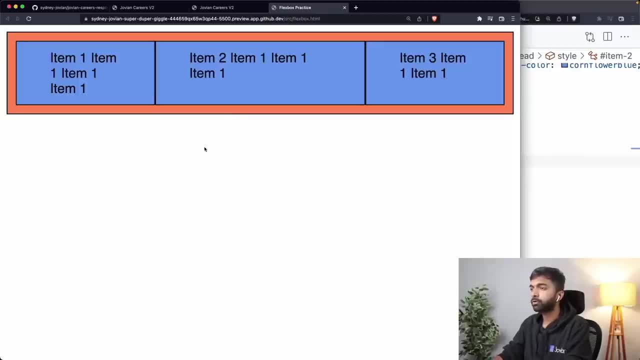 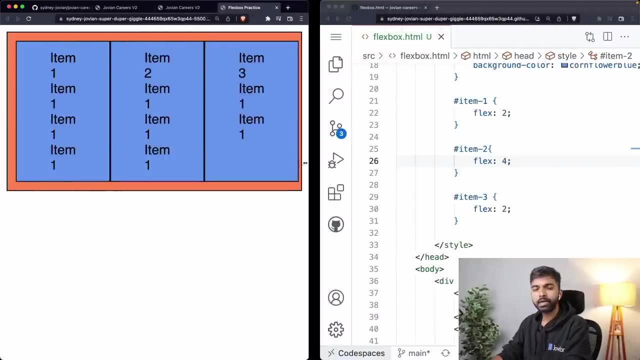 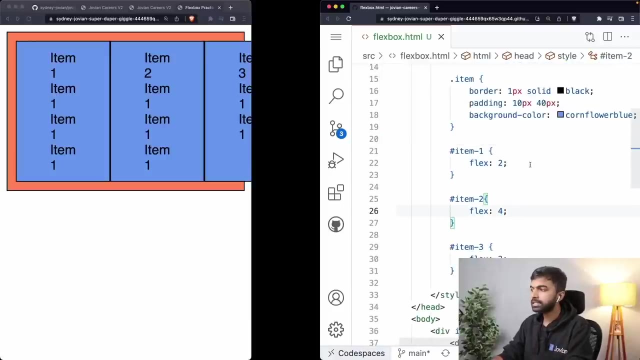 I can just specify something like this: Lex two, Lex four and flex flexed. And now These are automatically scaling, as I expect. So there is the base size that still applies, a very basic minimum base size. So when you do flex to flex for flex, to what that means is you're saying that the flex 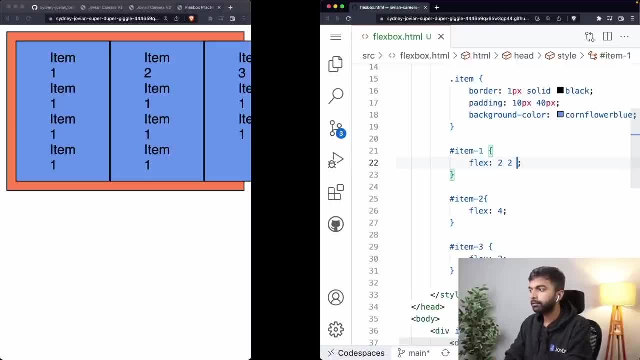 grow value is two, the flex shrink value is two, And then the flex while you is. or the flex basis value is zero or the minimum possible space. So normally you'll just end up doing this flex to, flex for and flex to, or setting some. 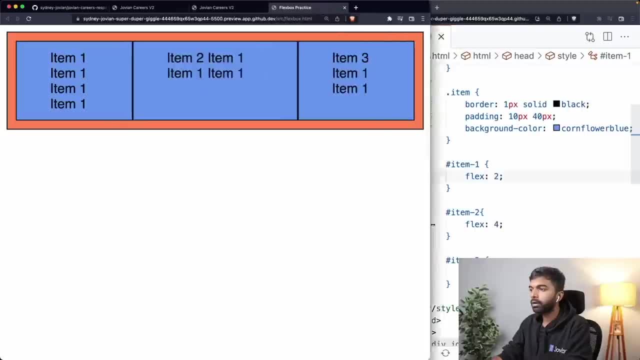 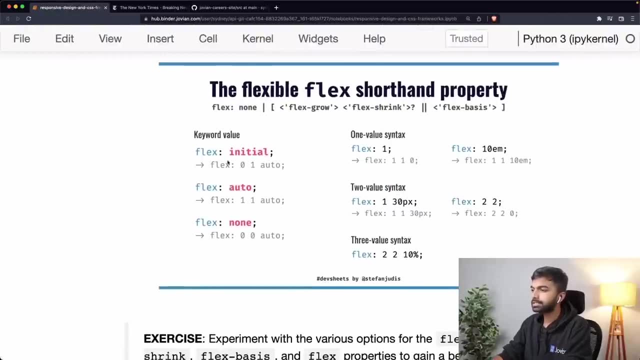 kind of a proportion between these flex items And that is how you'll use it. But you have a bunch of different ways to use the syntax. You can just set a single initial value, You can set it to auto, You can set it to none, which will just use zero, zero, four, zero, zero for each. 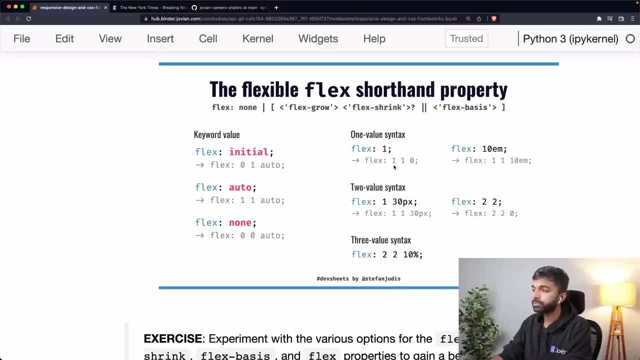 And you can just use a single value, one value syntax, like flex one, which is going to set it to one one- zero, or you can use a two value syntax, which is going to set it to one one and then maybe a specific base size of fixed base size. 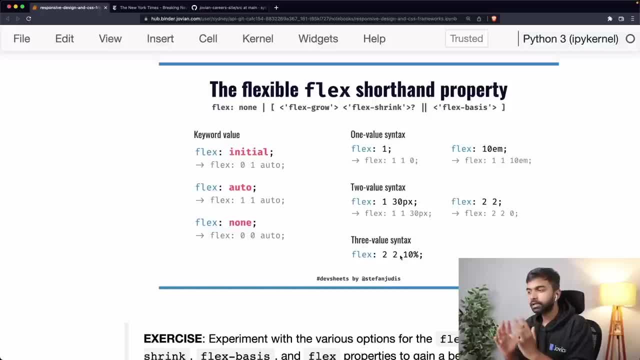 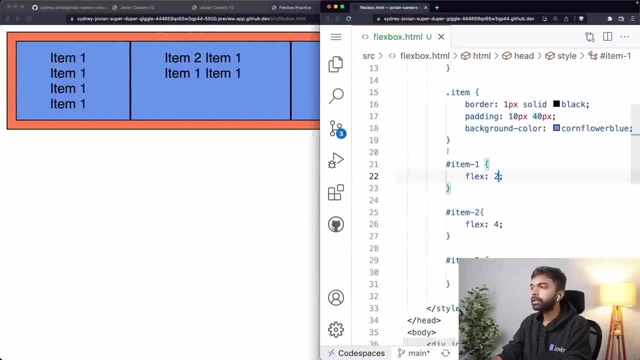 Or you can use a three value syntax. Okay, You can use a three value syntax which is going to use a certain percentage base size as well. So you have a bunch of ways to set the flex property. The most common use case of the flex property is something that I want to show you, because 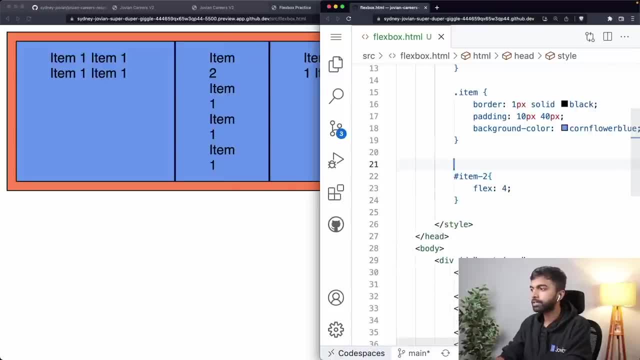 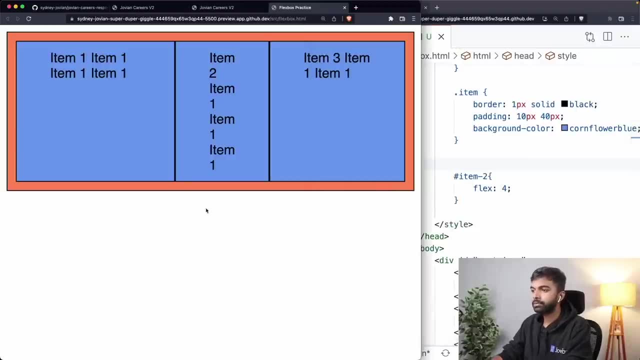 flex, grow, basis and shrink. I almost never use them because they never lay out the never that complicated that you need to use all these properties, But the most common layout that I use is that one of these needs to take up all the additional space. 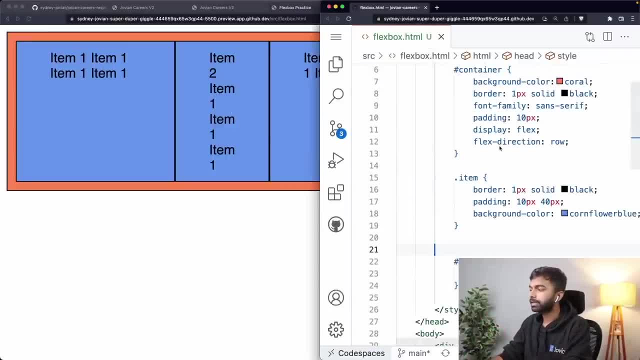 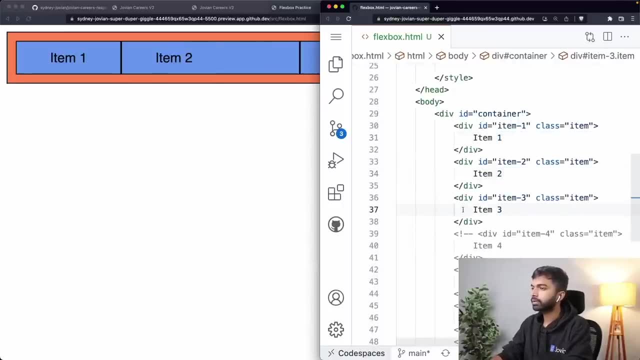 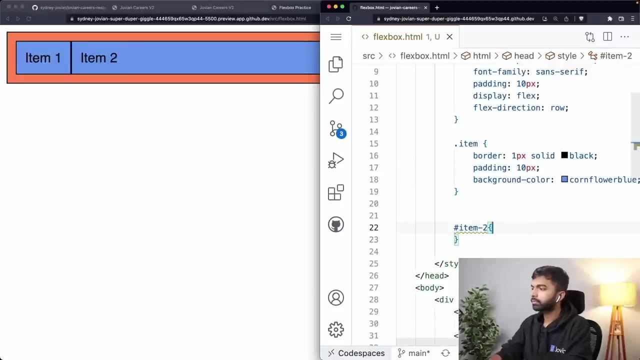 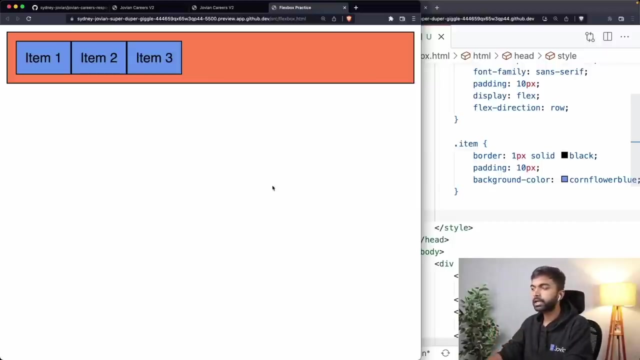 So you do not need to take up the additional space. in that case, I would do something like this. I would just go in, Let me just reduce the content a little bit and let me reduce the adding here a little bit as well. the most common use of the flex property, which is the flex grow, shrink and 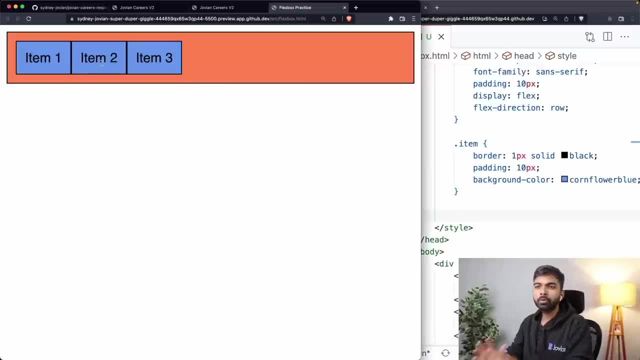 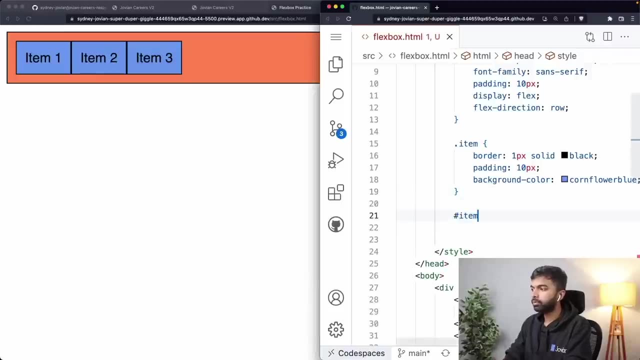 basis property is this: You want item two to take up all the space in between, No matter what the screen width is. So I would just go in into item two and I would say flex one, And just by doing that, just by setting flex one, item two takes up all the space in between. 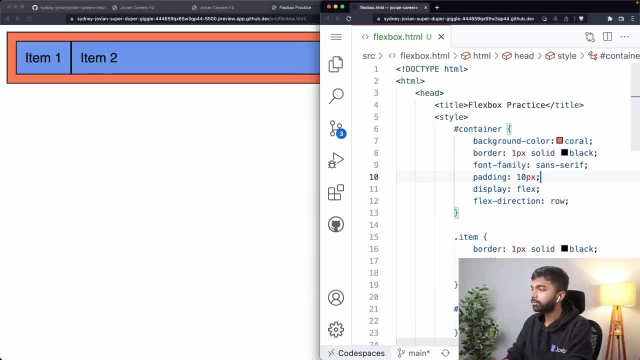 not just horizontally, but this can happen vertically as well. So let's say we have display flex and flex direction column, Okay, Okay, Okay. So let's say we have a height of 150 PX, or let's make that 250 PX. 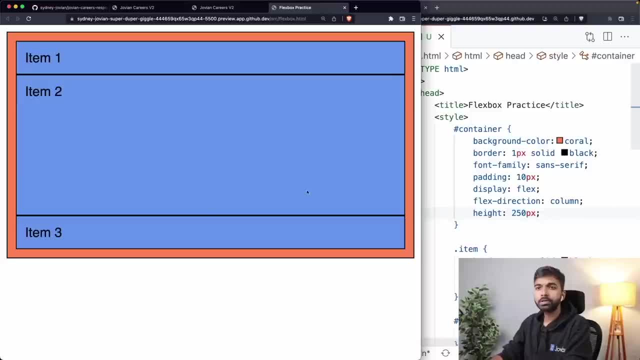 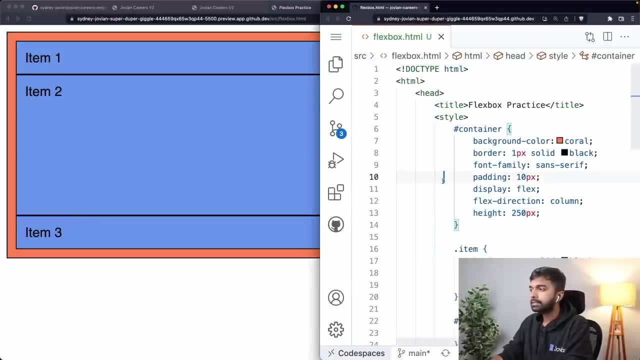 Yeah, So you can see here now we are taking up all the available space in this direction, right. And similarly, one other use case you might have is that I want item one, item two, to always have the same width. So let me just go back to flex direction row. 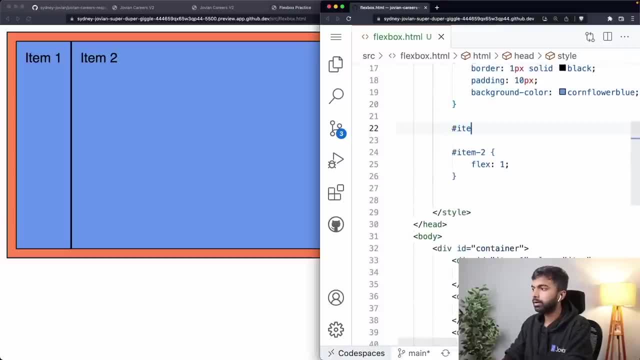 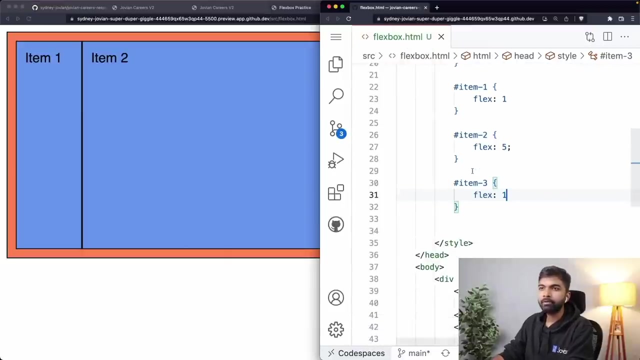 And let me just set item one, flex one, let me just set this to flex five or something like a very high value, and item three. Now you can see here that more or less item one, item three, are going to have similar rates, and we don't necessarily have to achieve it by setting these flex values. 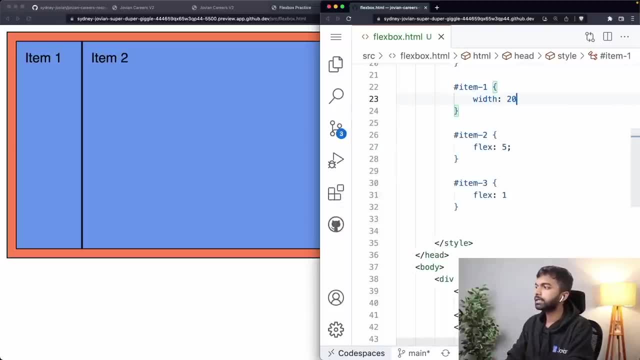 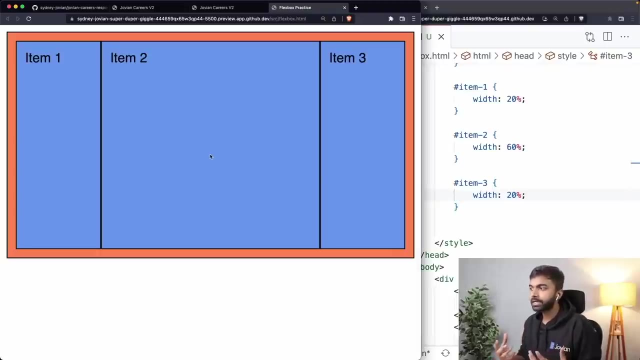 We can also just do these in this way. We can just say width 20% And width 60% And width: Okay. So this is the actual, real use case of the flex property, or why we use flex box: because we want to achieve a certain set of widths. 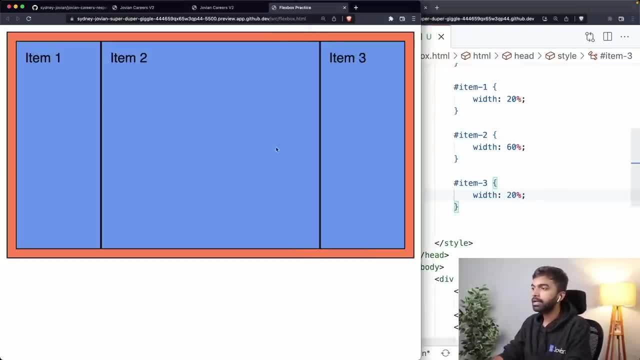 This may be our main content, This may be a left content, This may be a right content. Now, all of that. of course, when we are using the flex property under the hood, it's using flex basis, Flex grow, flex shrink and all that. 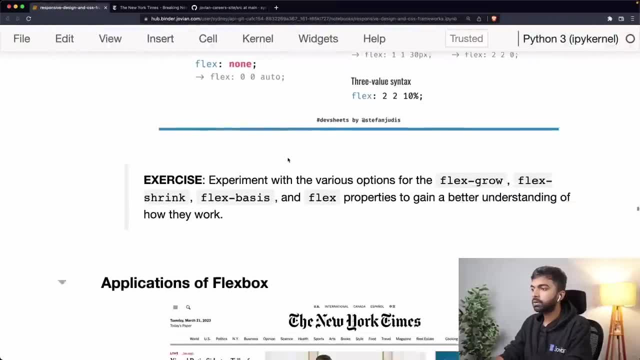 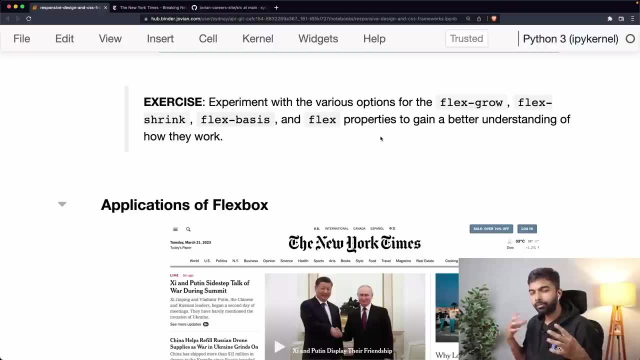 But I just use the flex property directly. Okay, So, experiment with the various options for flex growth, flex shrink, flex basis, But don't stress if they don't make a lot of sense, because there are certain edge cases, certain special scenarios which you may not be able to keep in your head. 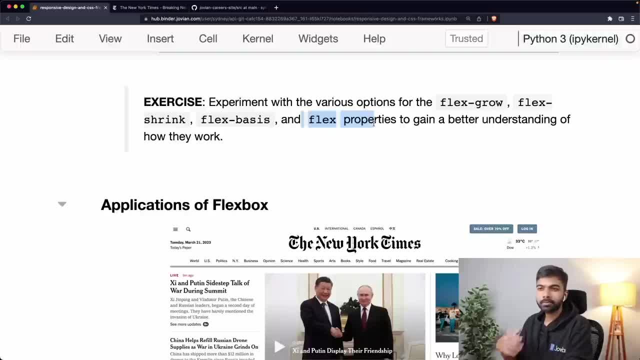 You can always just look them up. The key is maybe just to use the flex property and try to get what you want, And the most common use case is either setting flex one to expand a certain div to take up all space, Or using flex one on a couple of divs to maybe make them roughly equal width. 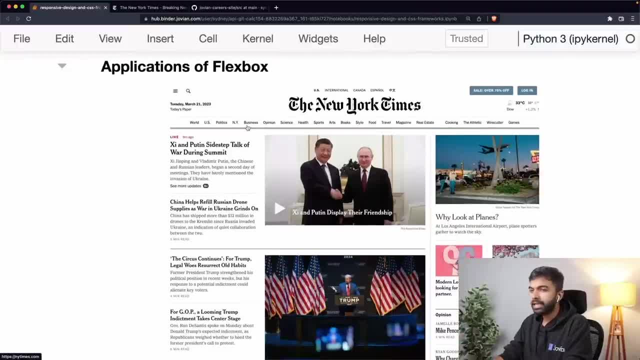 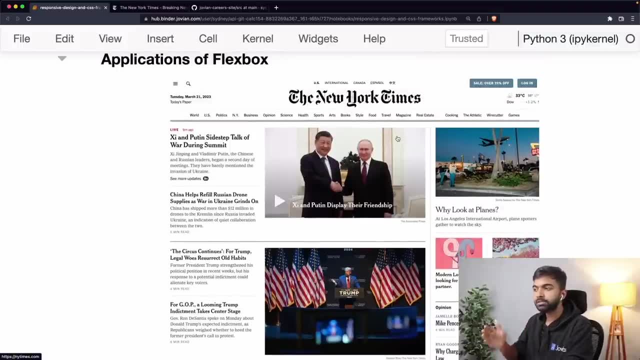 Okay Now, flex box has many applications in all kinds of web design. As you can see for the New York times website, this kind of a layout is achieved and made responsive only using flex box. It is used to create responsive layouts. It is used to create certain grid systems as well. 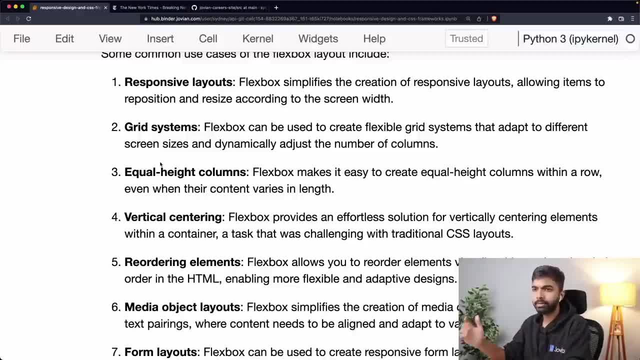 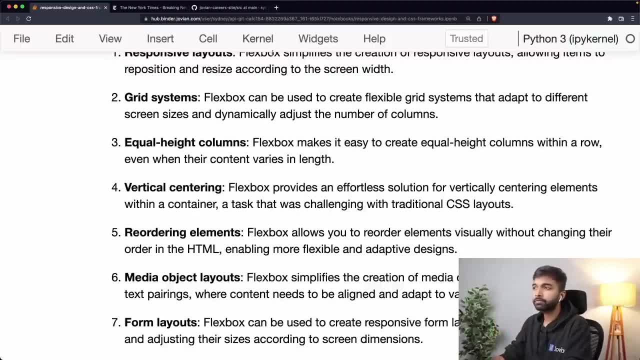 There's a separate layout called the grid layout, which we have not covered today. We'll maybe try and cover at some point. Okay, It is used to create equal height columns. Let's say, you want to have maybe a bunch of cards showing side by side. 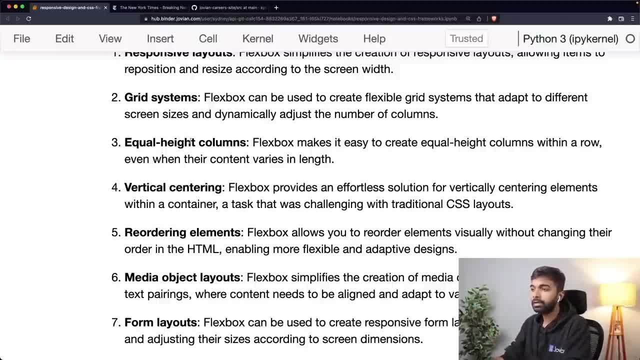 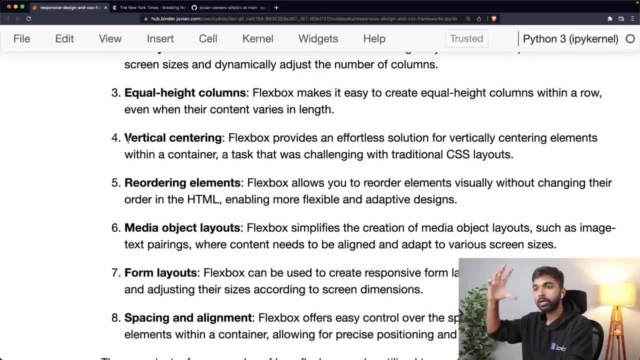 All of those cards should have equal height. That is something that you can create using flex box. It is used to perform vertical centering. Let's say you want to center a div vertically on the page or vertically inside another div. The way you do it is simply by setting flex direction. columns justify content center. 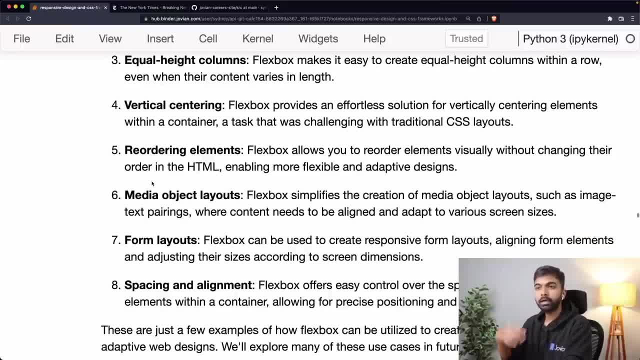 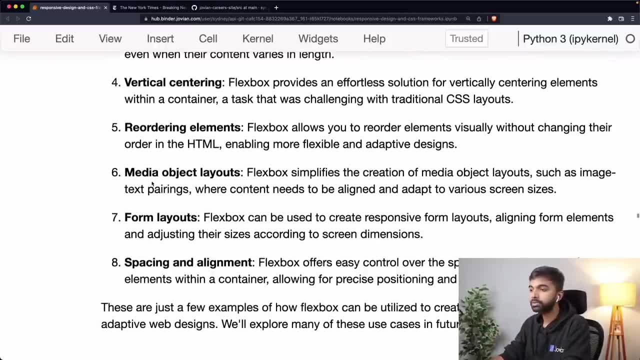 or flex direction row- align item center. It is used for reordering elements. Sometimes on mobile You can use the left to write a certain layout and on desktop you want to reverse layout. So that's what you can use it for. It is used for maybe showing image and text side by side. 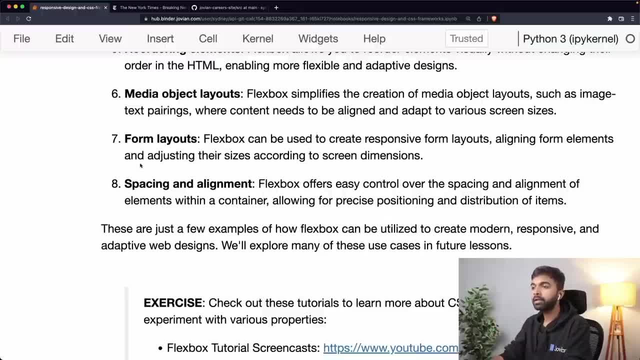 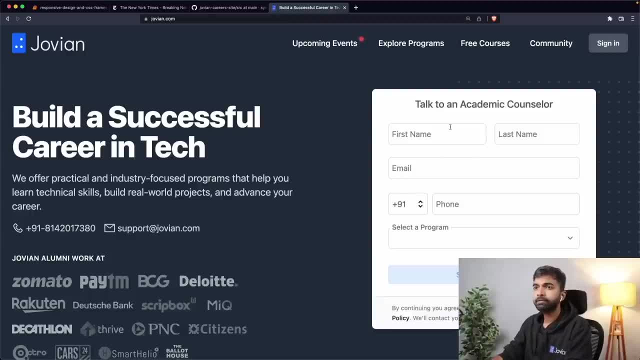 It is used for creating responsive forms. Let's say, you have a form where you have a first name, last name. an example of this can be seen on the Jovian website, So you can see that first name and last name are side by side. 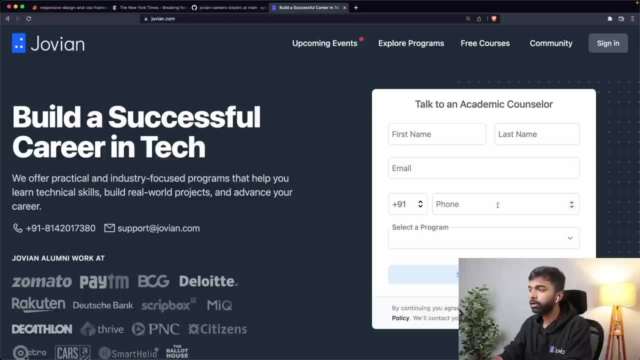 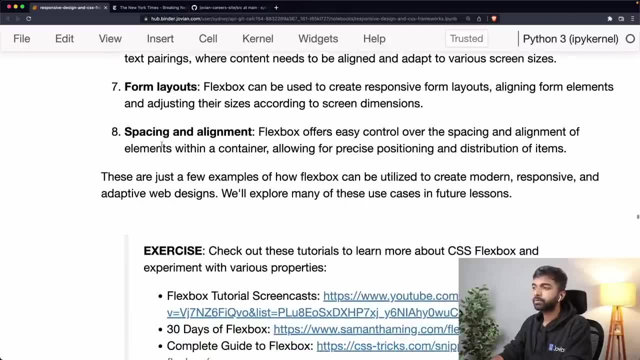 And then again you have email, and then we have phone number and you have the country code and phone number side by side. Then you have again the program. So all of this is achieved Using flex box and it is used for ensuring spacing and alignment, making sure that something 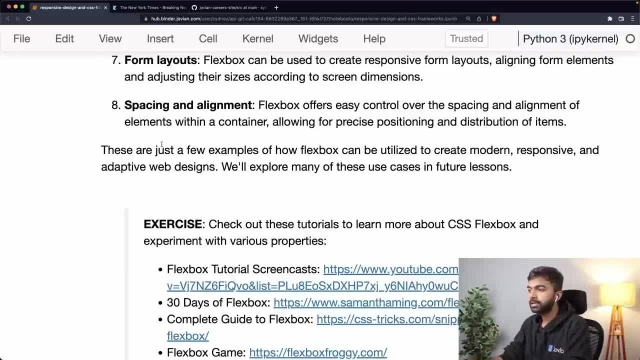 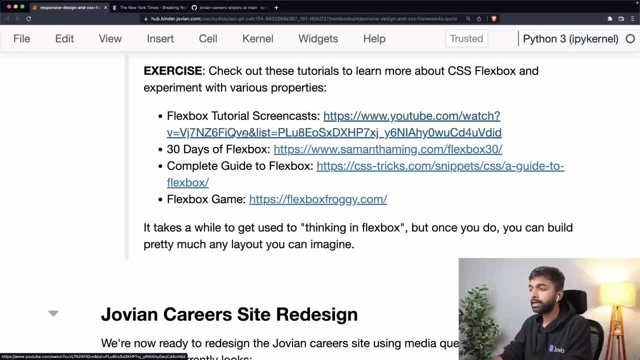 takes up the entire space making sure that two divs are the same size, And there are many tutorials you can go through. The more practice you get with flex box, the better you will get at it. specifically, I would highly recommend the series of screencasts by best boss or what the flex box it goes. 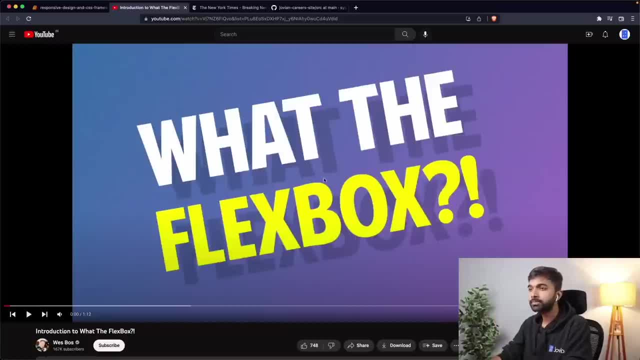 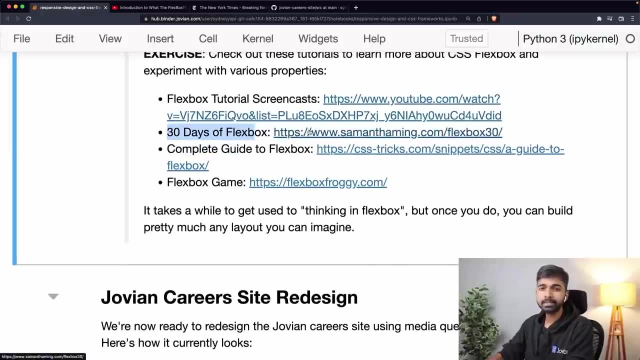 into each flex property, And then it shows you a bunch of specific scenarios as well, And I would also highly recommend you to check out Okay, 30 days of flex box, which is again a series of tutorials that you can follow along day. 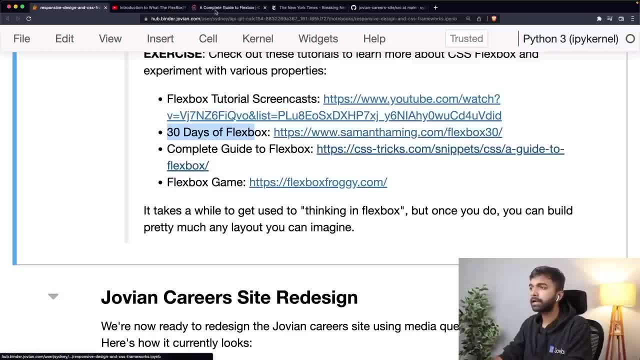 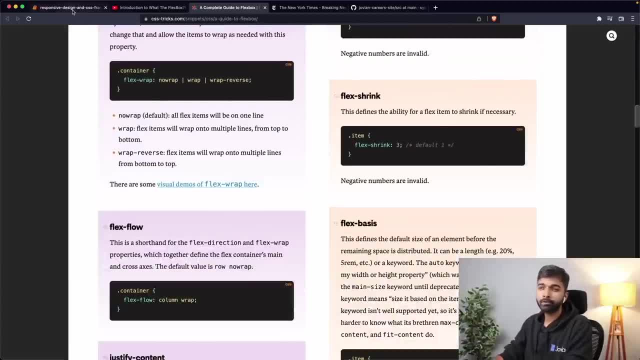 by day And there is just for reference. there is this complete guide to flex box that you can always check out. This contains a bunch of visuals and it contains information about each property. that you don't have to remember this. I always look this up. 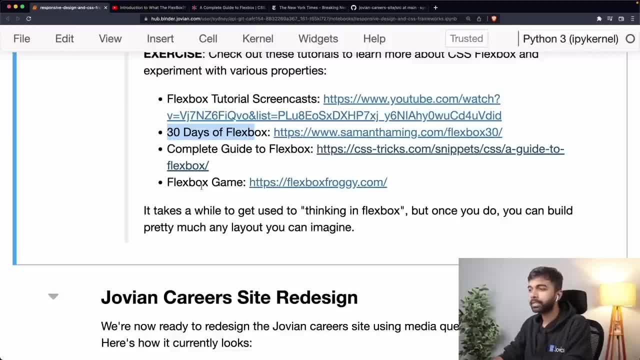 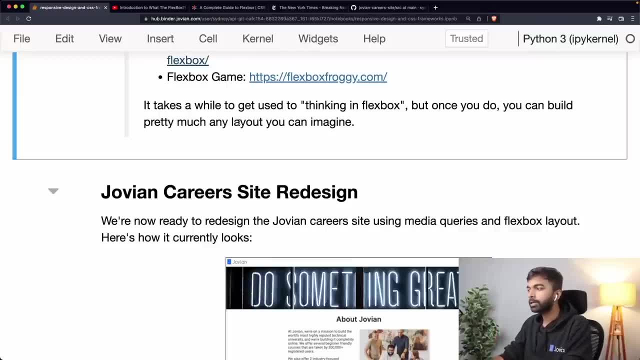 I never remember this, even after using this for probably 10 plus years at this point. Okay, But it takes a while to get used to thinking in flex box, But once you do, you can build pretty much any layout that you can imagine. 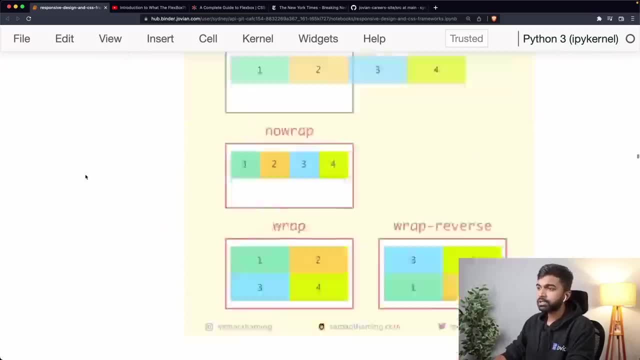 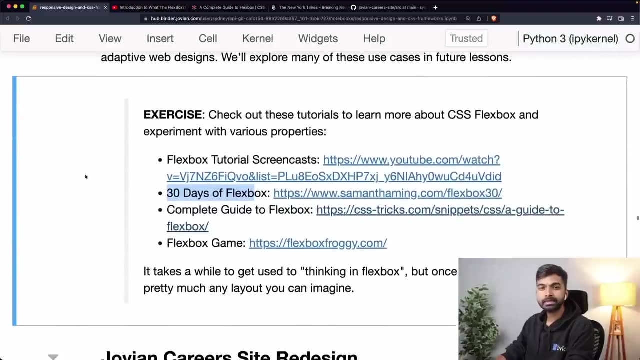 Right. So the last thing I'll say about flex box is that it's powerful, but because it is so powerful, it is also somewhat confusing. It takes a while to get used to it, but don't give up, Don't run away from flex box. 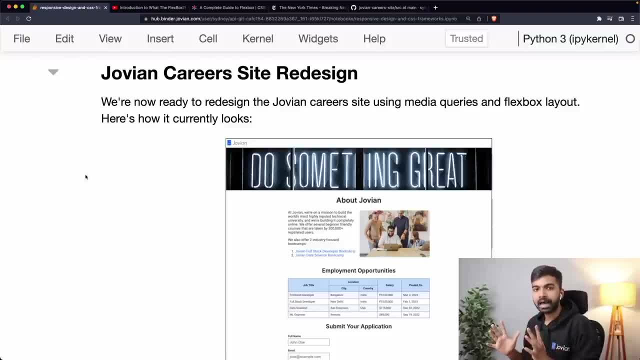 Just limit your usage to basic flex direction, flex, wrap and align items and justify content And maybe every now and then use the flex property. So let's now go ahead and redesign the Jovian career site. So this is what it looks like on desktop. 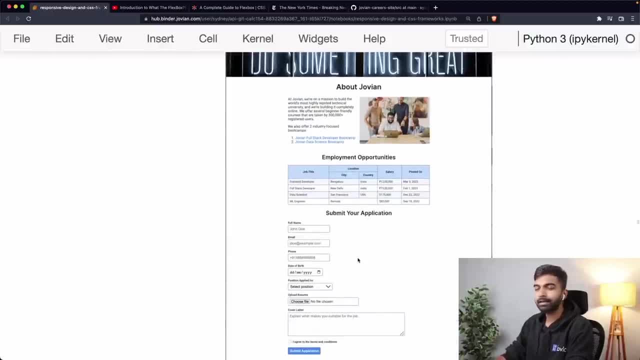 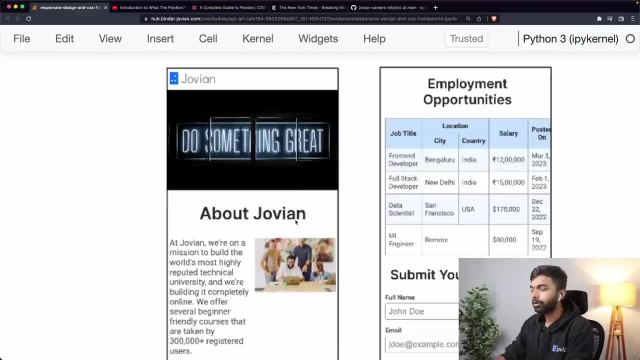 I think it looks fine on desktop. for now, We don't need to really redesign anything here, but we do want to redesign it on mobile, because on mobile it definitely doesn't look good at all. So we want to do something with the mobile design and we are going to follow these steps. 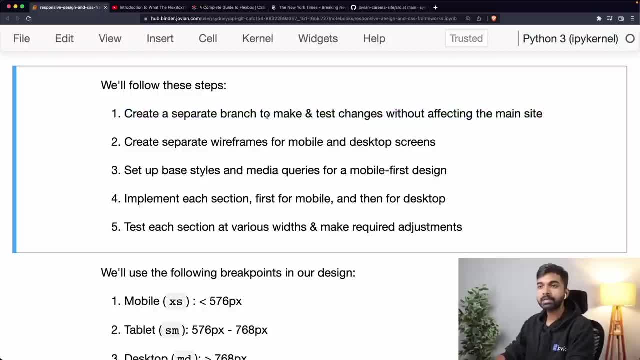 What's? we're going to create a separate branch on our code space. Remember, we don't want to affect the main site when we are making changes, when we are experimenting, So we're going to create a separate branch and test our changes there without affecting. 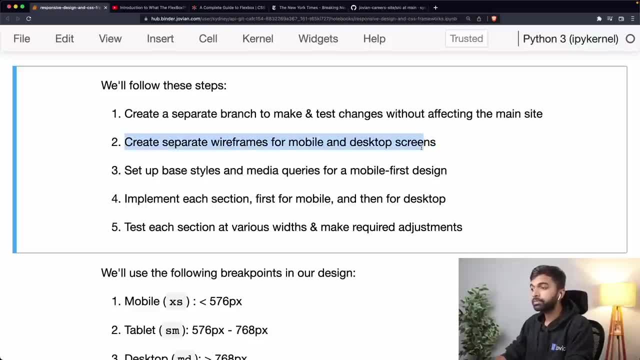 the main site. Then we are going to create separate wireframes for mobile and desktop screens. Then we are going to set up base styles and media queries for mobile first design. Then we're going to implement each section, first for mobile and then for desktop. 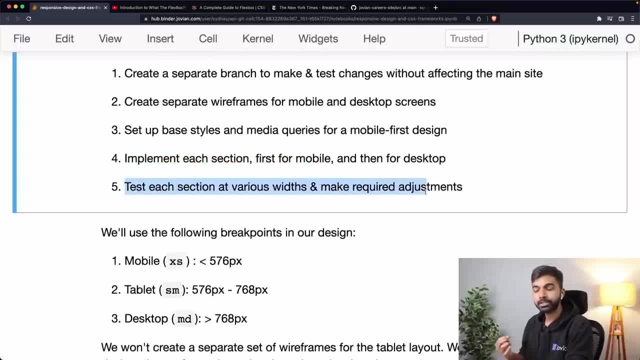 Then we're going to test each section at various widths and make required adjustments And finally we're going to create a pull request. We're going to review that pull request, review the preview deployment and then merge it back to the main site. 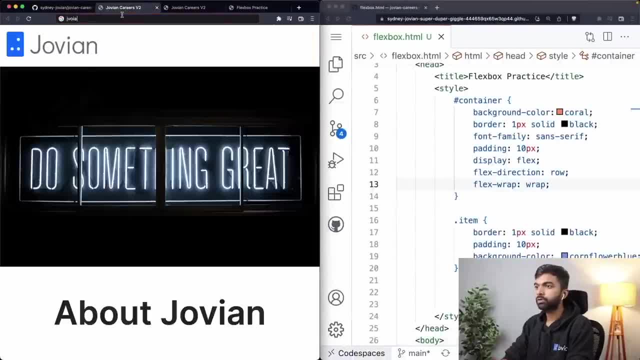 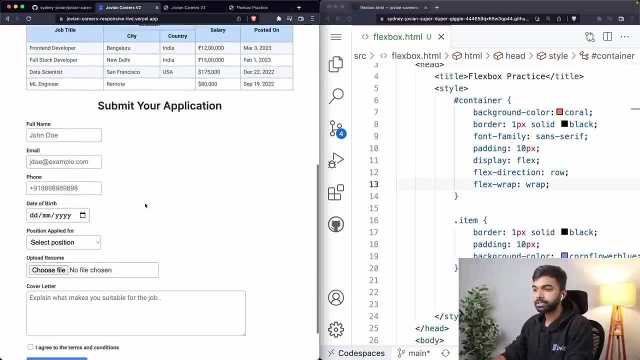 Okay, So the main site, which is jovian-careers-responsive-livevercelapp- This is going to remain unchanged till we merge our pull request, right. So this is what the common practice is: that you have the main site. that is running. 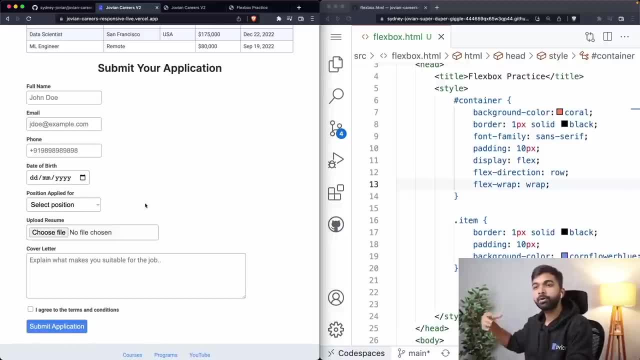 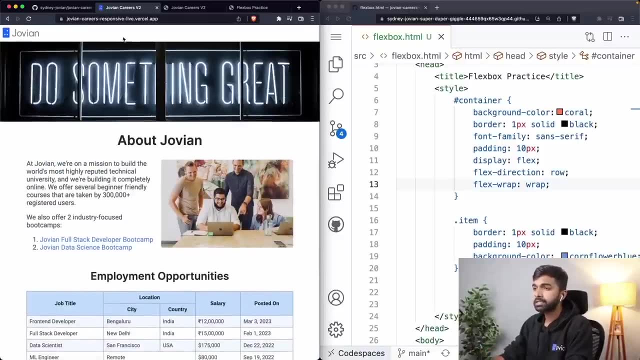 Then you create a branch work on your feature And once the feature is reviewed and tested and merged back, then this will automatically get updated because Vercel will do an automatic deployment for it. Okay, So this is our main site. We're not going to affect that, but this is our preview site, which we are looking at. 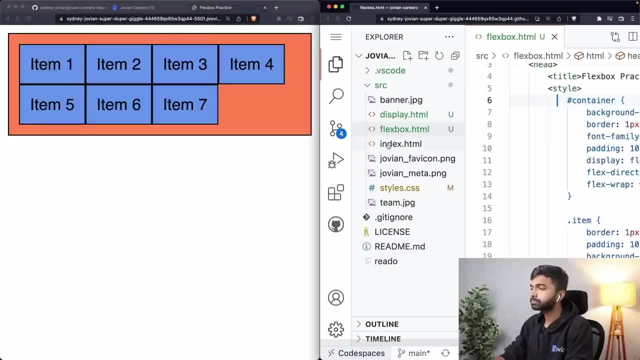 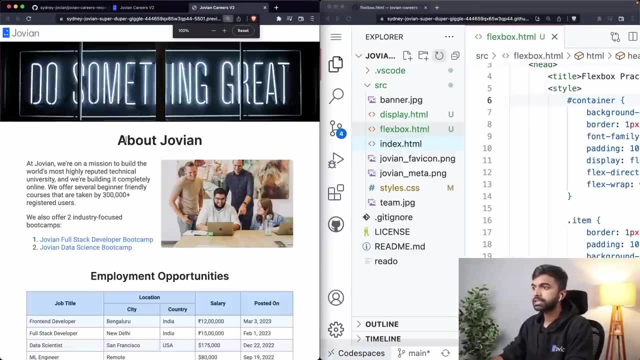 here. Let us just open up indexhtml. open with live server. put that in here. So this is our preview site. Let me just set it to a default width. So this is what it looks like on desktop. This is a hundred percent width. 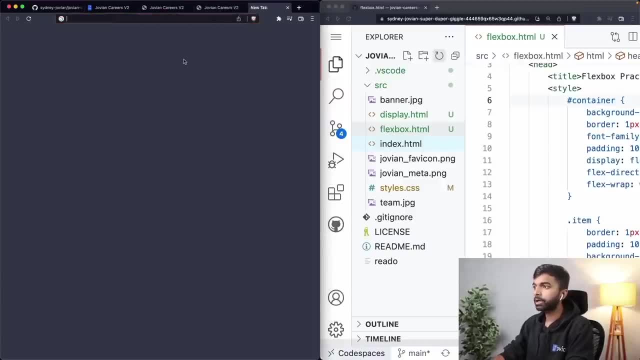 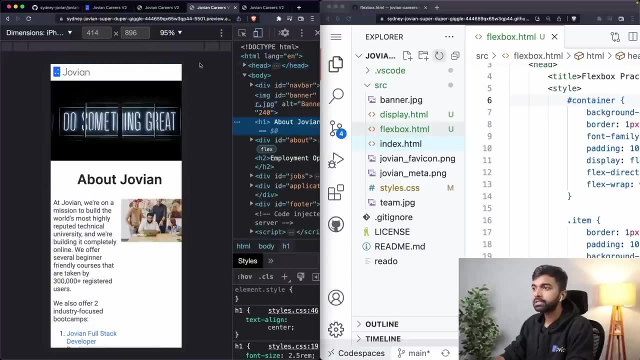 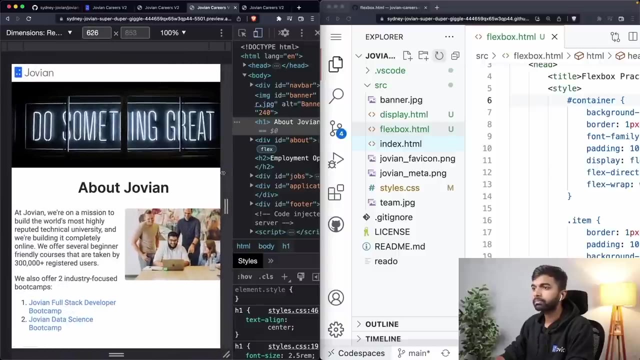 Let me just open the same page up in a couple of other browsers as well. Okay, Okay, Okay. So we have different devices in each case, but here I want to study its width on the tablet. Let's say, maybe a tablet would be about 700 pixels. 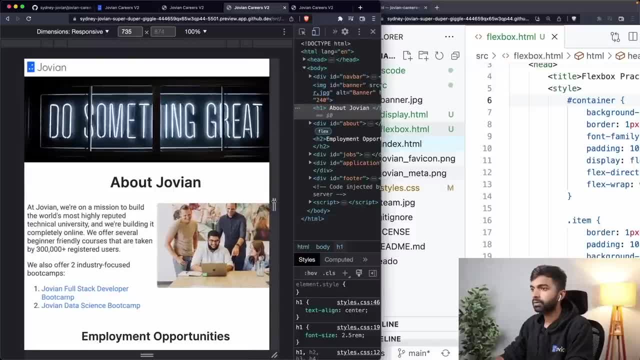 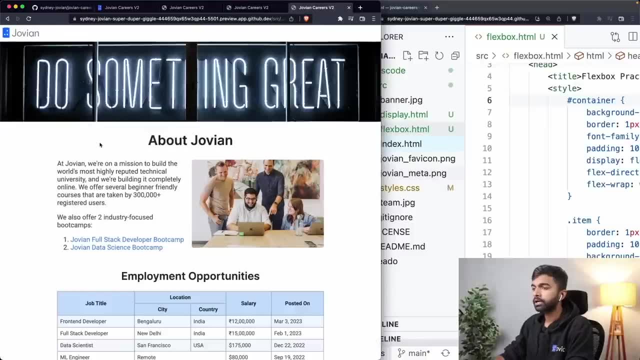 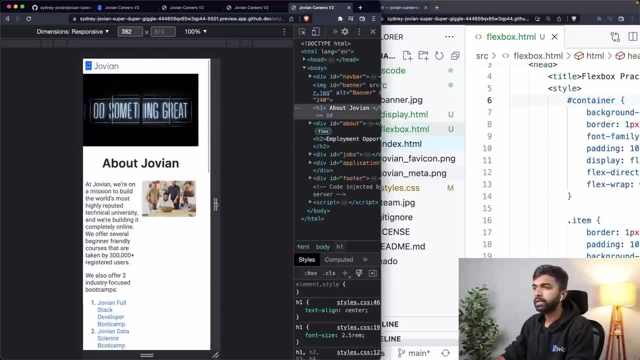 A little bit here. Yeah, So about 750 pixels, I believe, would be a tablet layout, And let us also create a mobile layout here. So we're going to look at a mobile layout as well. Well, let's design around 300 and maybe around 400 pixels. that is what most mobile layouts. 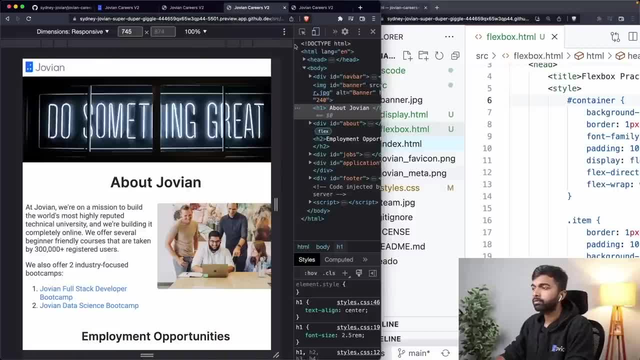 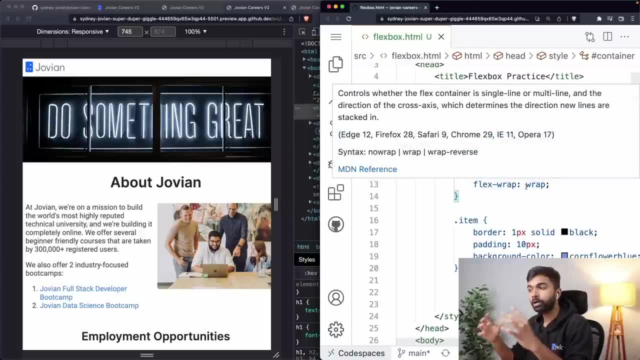 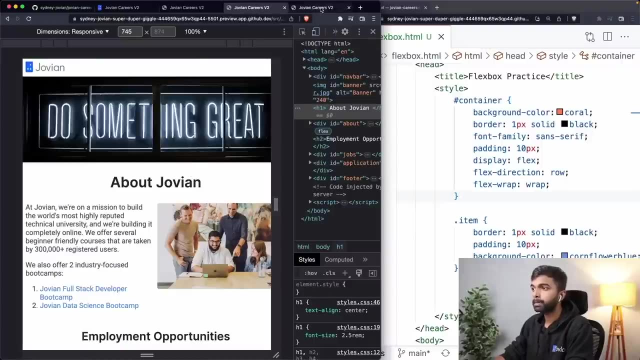 are around. okay, now we have for our code space, for our indexhtml, which is running using the live server extension. so this is all the preview of what we are doing on our code space. we have the mobile layout here, we have the tablet layout here and we have the desktop layout here and we're going to start. 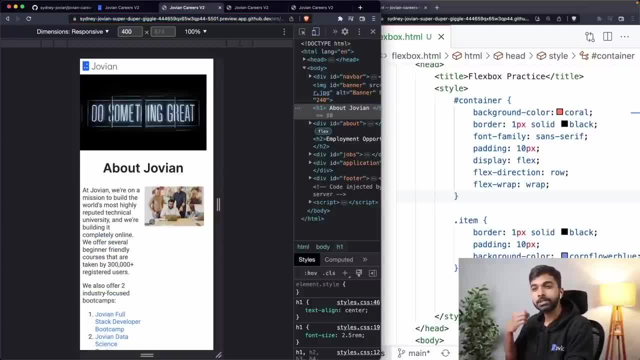 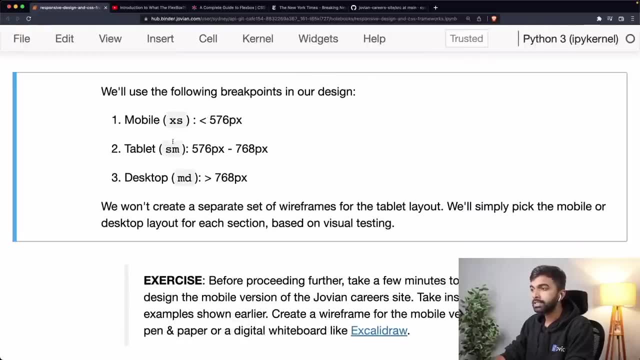 with the mobile layout. we're going to do a mobile first design and then we're going to slowly improve that layout to account for tablet and desktop as well. okay, so we're going, we're going to use these breakpoints under 576 is going. 576 pixels is going to be a mobile layout. so this is about 400, that's. 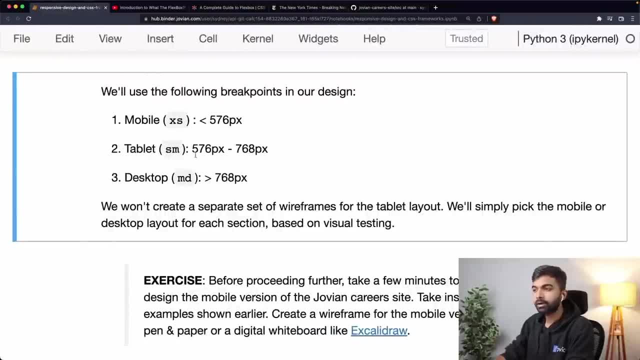 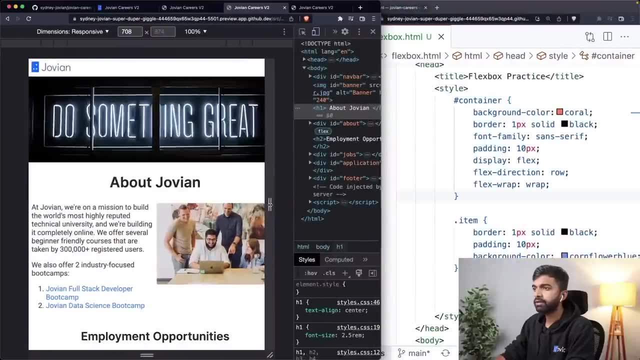 mobile. under 768 pixels and above 576 is going to be a tablet layout. I believe we've set this to about- yeah, we've set this to about 7. let's set it to about 740. yeah, so that's in our, that's in the tablet range, and we can always go left. 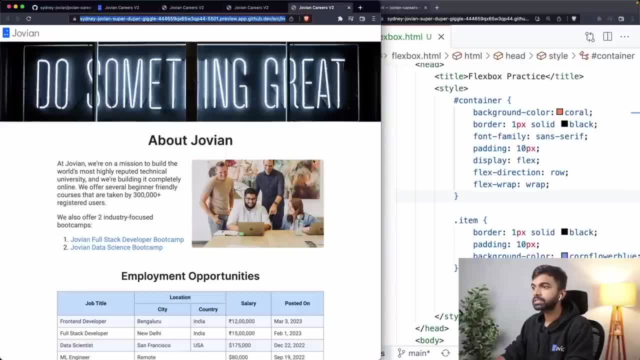 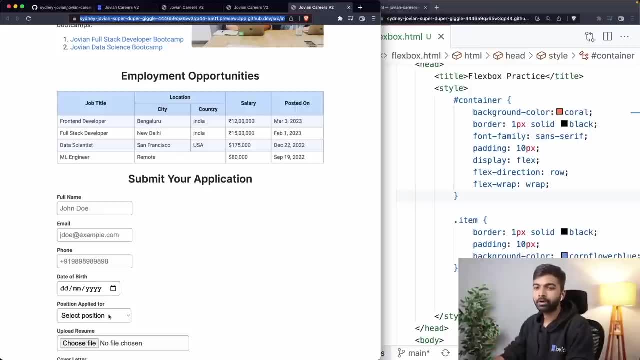 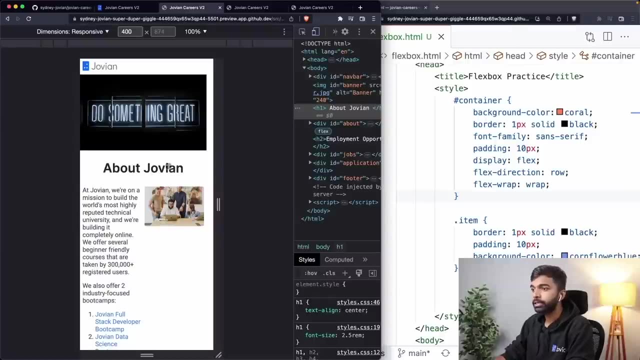 and right and we can shift things, and greater than 768 pixels is going to be a desktop layout, which is what this is, and of course, we can also then consider large desktops, etc. for now, I'm simply not considering those, okay, so let's get started step by step, slowly. 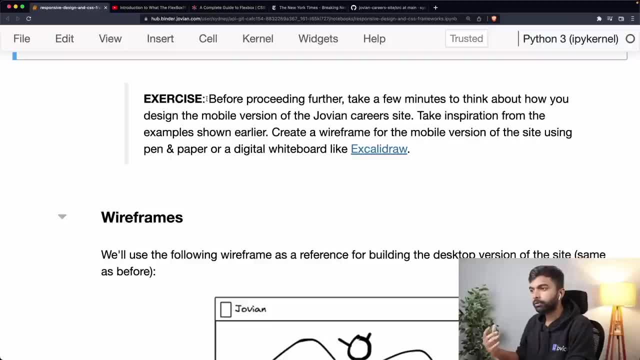 we proceed. I would encourage you, as you're reviewing this, to pause, take a few to think about how you would design the mobile version of the job in career site and take inspiration from the examples that we looked at earlier and maybe try to create a wireframe for. 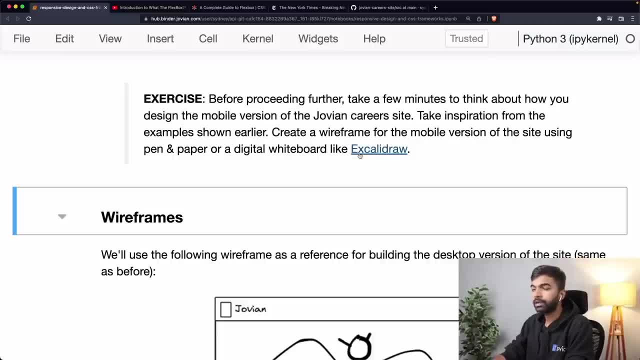 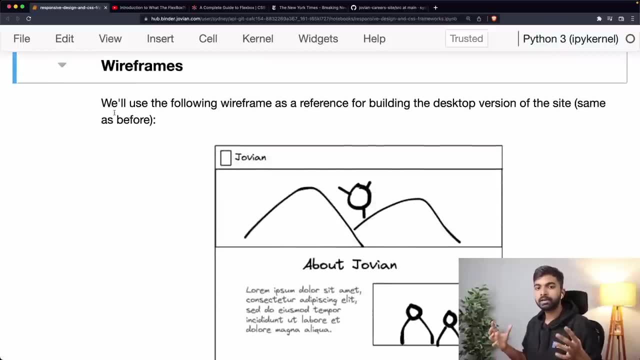 the mobile version of the site on pen and paper or using a digital whiteboard like xcalidrawcom. but here is the wireframe that we are going to be using now. typically, a design mock-up that is given to you is going to be given for mobile, tablet and desktop. similarly, we can try creating. 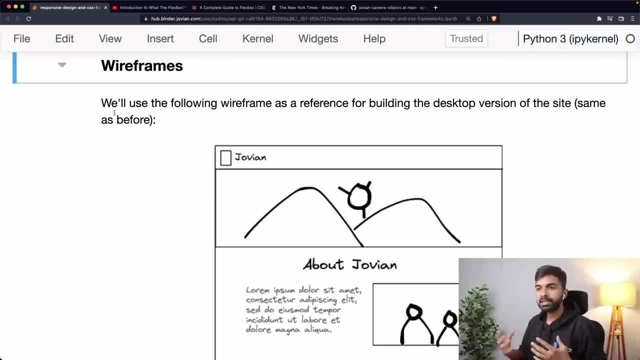 my frames on mobile, tablet and desktop. but just to keep things simple, we are just going to create a mobile wireframe and a desktop wireframe. excuse me, we're going to keep things simple: use a mobile wireframe and a desktop wireframe. and for tablet, we will just approximate and maybe pick some. 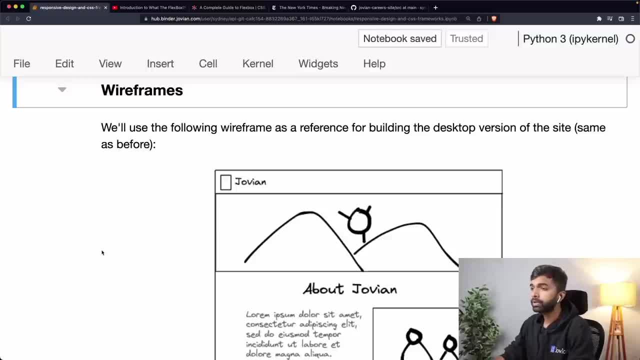 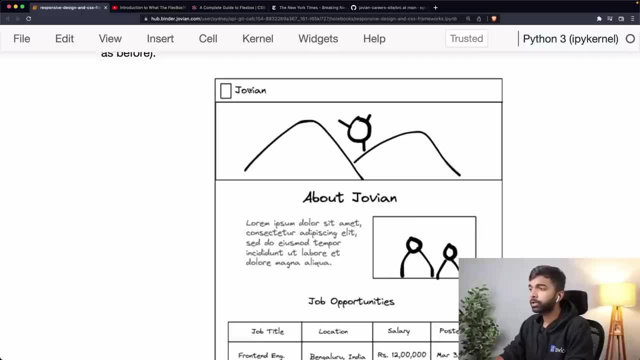 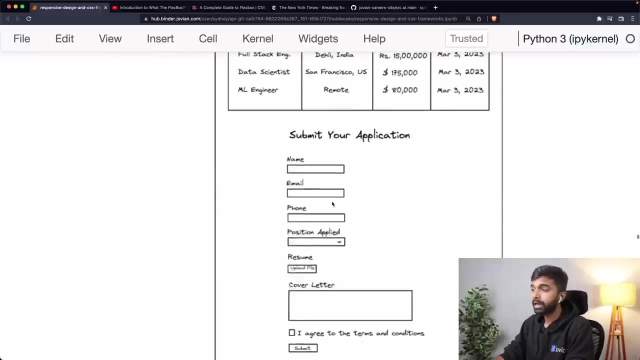 elements from the mobile and some elements from the desktop. okay, so for the desktop view, we are going to use the same layout that we had earlier, so which is the jovian logo here at the top with the jovian text, then an image here, the about jovian section, the job opportunities table and the submit your 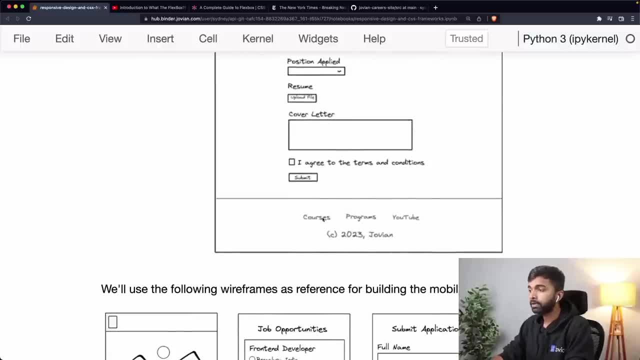 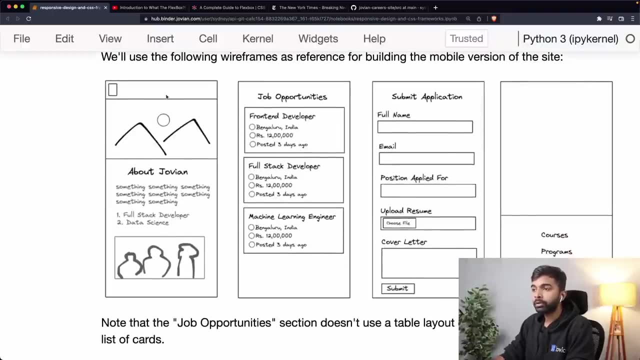 application form and then there is a footer at the bottom with a bunch of options, courses, programs and youtube on mobile. here is what we are going to do. we are going to use a navbar, but in the navbar we're not going to show the entire jovian logo. we're just going to show the jovian icon. 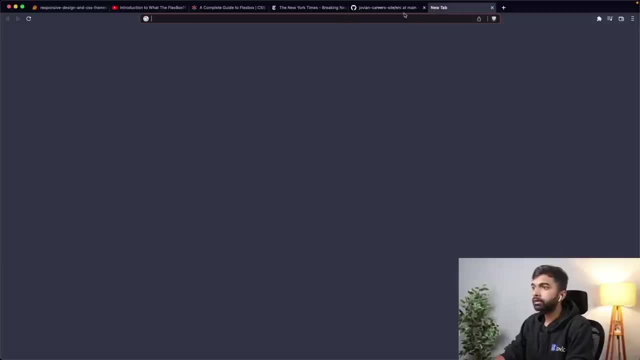 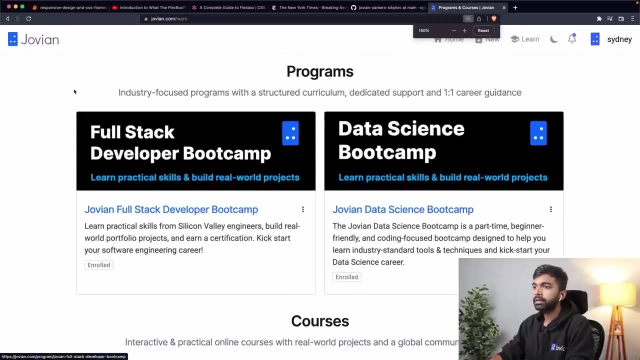 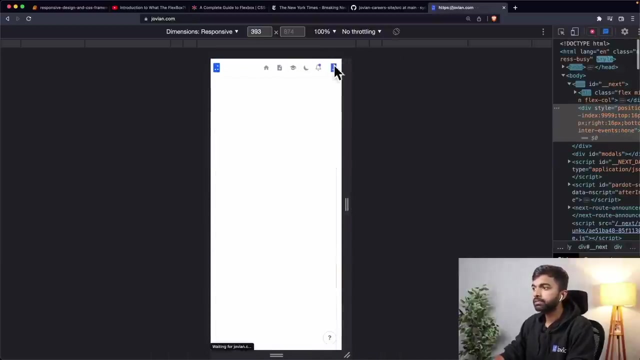 okay, this is a common practice on mobile that you often just show the icon. so i'll just show you an example of this. let's say i go to joviancom learn, zoom in here a little bit and if i go into the mobile view here you can see that at this point we only show the icon because we often have a bunch of things on. 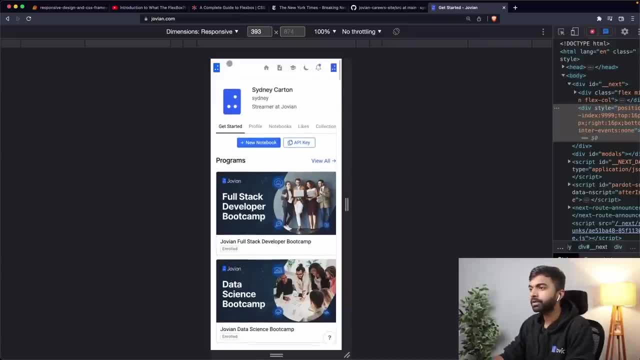 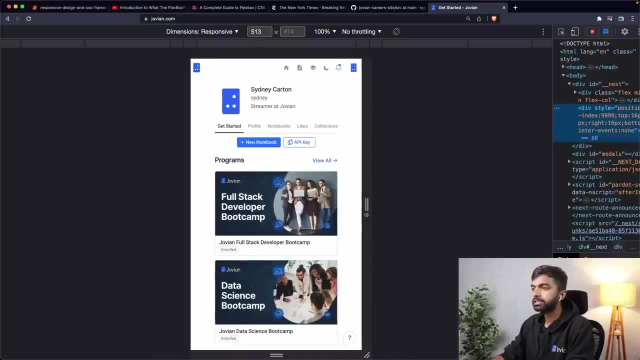 the right as well. this is the profile icon, which also happens to be the jovian logo. but yeah, we only show the icon on the mobile and we also maybe change the layout slightly on mobile, as you can see on the jovian platform as well. okay, so on mobile we're going to show. 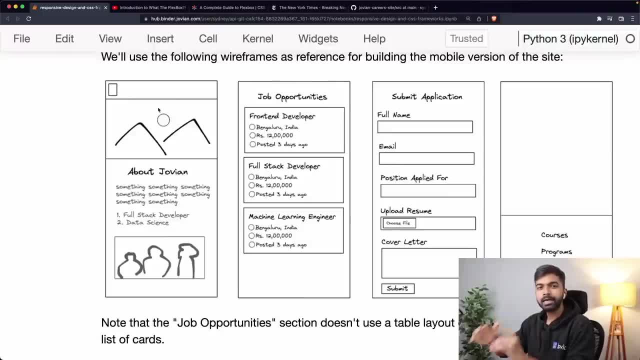 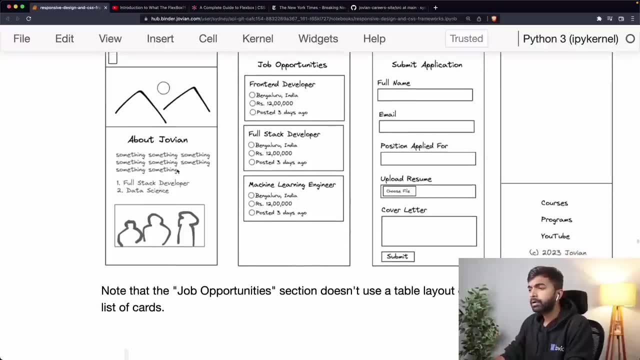 the icon. we are going to show the image, but we are probably going to reduce its height a little bit not to ensure that not to take up the entire page, otherwise it might just take up a lot of space. then we are going to have this about jovian section, where we are going to have this: 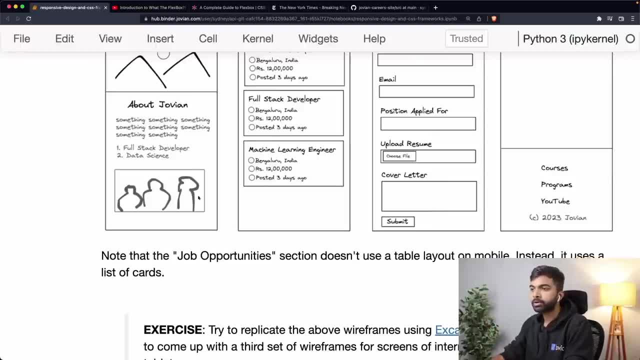 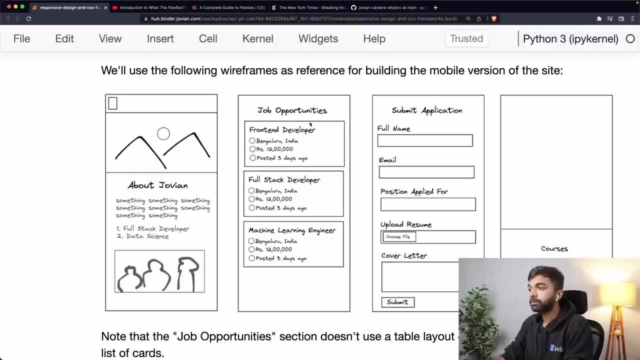 description and we are going to move the image below, and so the image is going to remain below, and i think i'll use the same layout for tablet as well. then we are going to have job opportunities, but this time, for job opportunities, we are going to use a list or maybe a bunch of divs, so we are 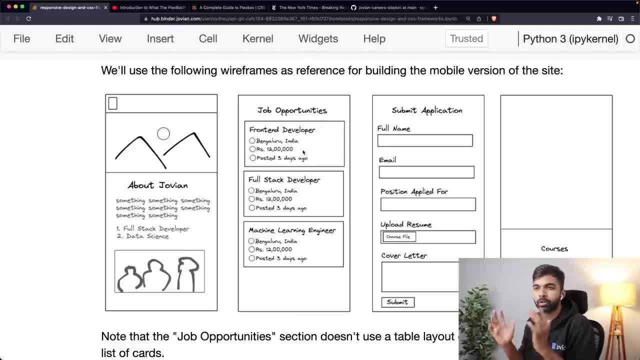 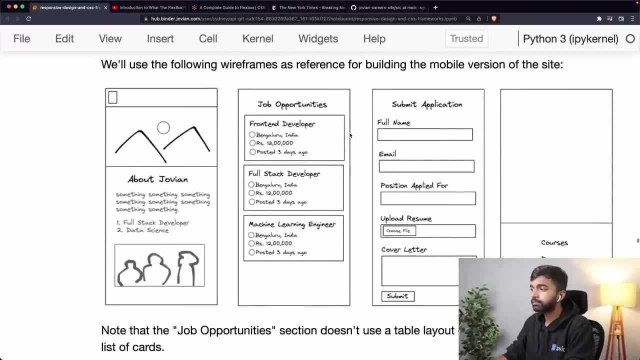 going to show these cards instead of actually showing a table, because on mobile viewing a table makes sense, but on desktop we are still going to use a table, so we're going to see how to achieve that. then we have this layout for application. so on mobile it's a nice idea to maybe just 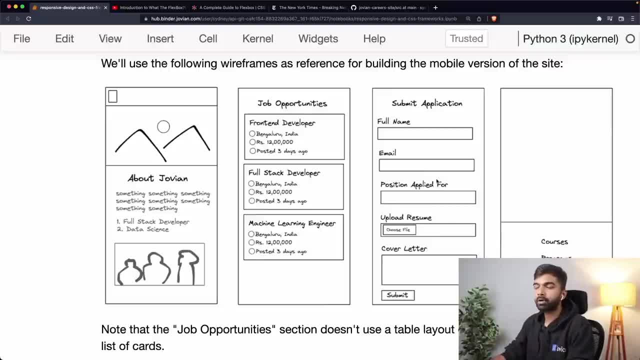 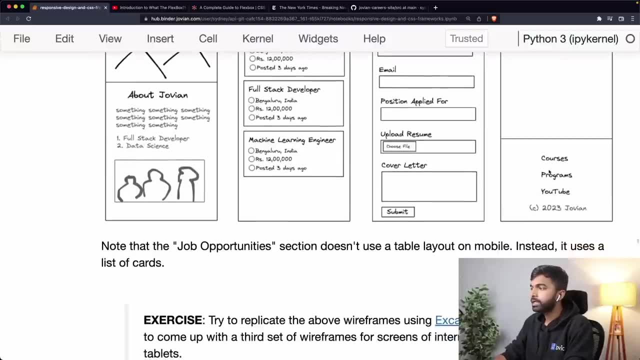 make all your inputs full width, so just let them occupy the full width of the screen and we have this upload resume cover letter button as well. and finally, for the footer, we are simply going to show the options one below the other, unlike on desktop, we are going to show: 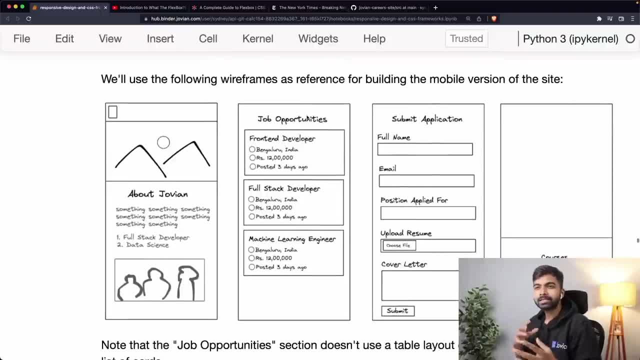 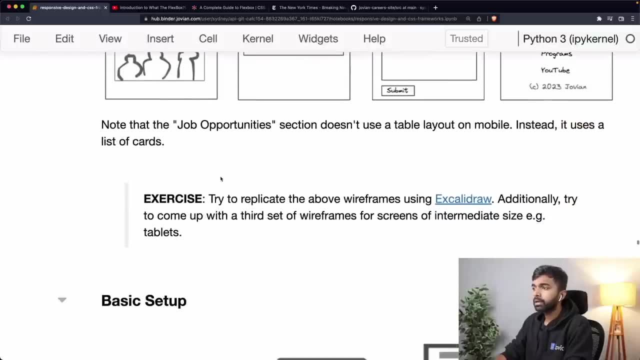 we are going to show the options side by side, okay, and we'll decide how to change these layouts for tablet as well, but these are the two layouts that we are working with, okay, and specifically, the job opportunities table is going to be the real challenge, because it doesn't have a table. 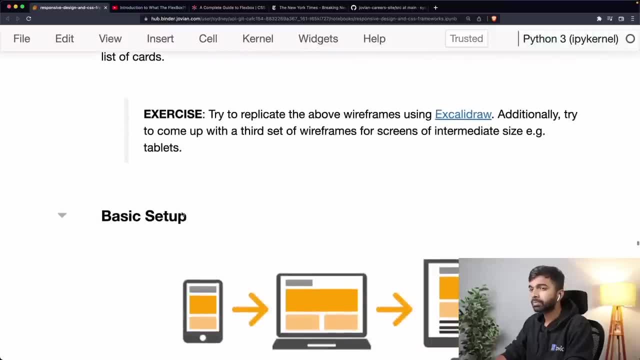 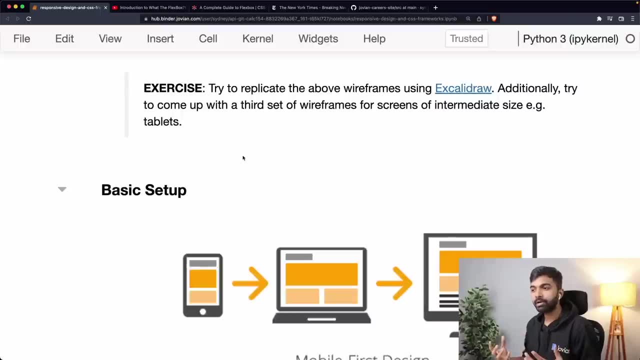 layout on mobile. it has a list of cards, and i encourage you to go ahead and replicate these wireframes on your own. wireframing is a very useful skill for a web developer. before you can go in and start coding the website, you should have a very clear idea of how it's going to look. 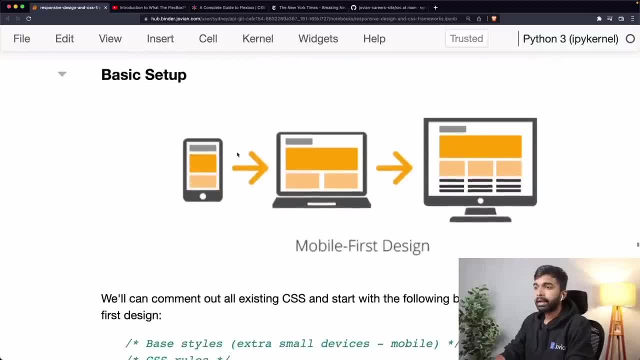 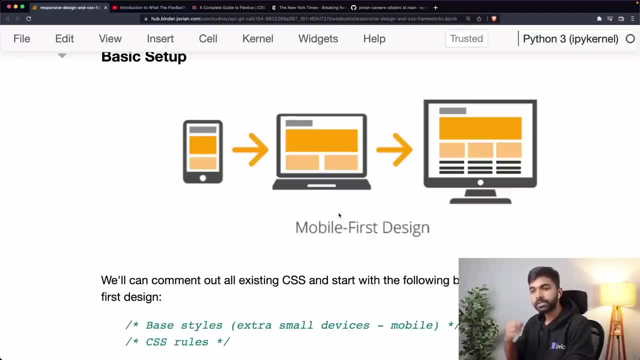 at the very least using these rough wireframes. and, as i've said before, we are going to follow a mobile first design, which means we are going to first set up css styles for mobile section by section, and then we are going to enhance the css styles for tablet and for desktop and maybe even for smaller, uh, for larger screens. okay, so for that. 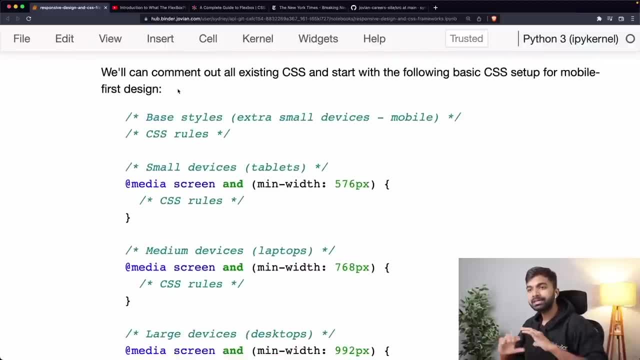 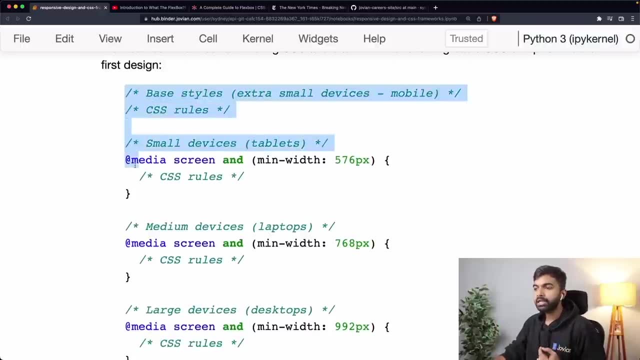 here is how we can begin. we can begin by commenting out all the existing css and just rebuild the page right from scratch, and we'll just put in a bunch of media queries at the beginning, okay, so first let's comment out all the css. let us open up stylescss here. 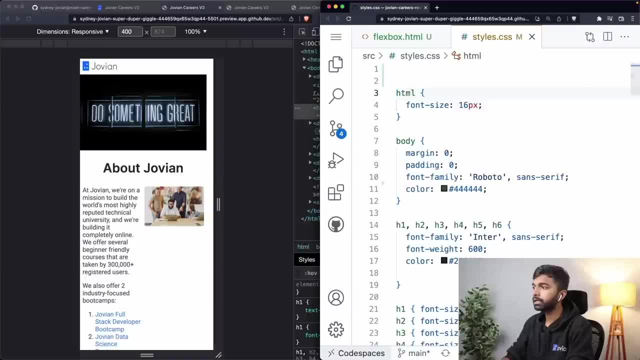 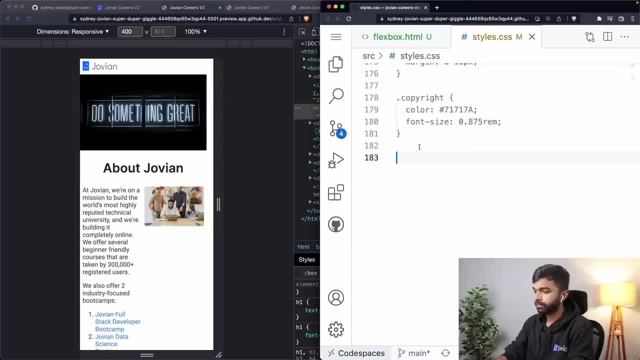 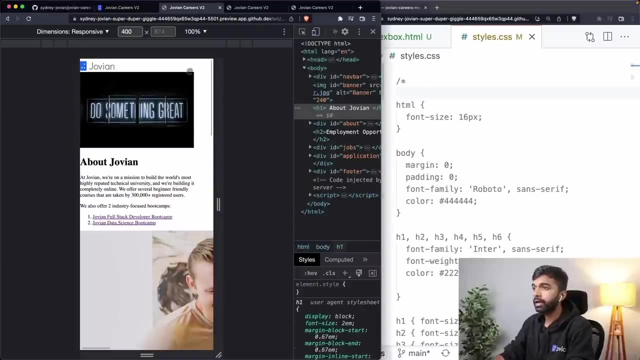 let us comment out all the css. the way we'll do it is by adding this star slash star at the top and then adding a star slash at the bottom. okay, so you added slash star at the top and star slash at the bottom and now if we reload our pages, we can see that all that, all the css, is gone. 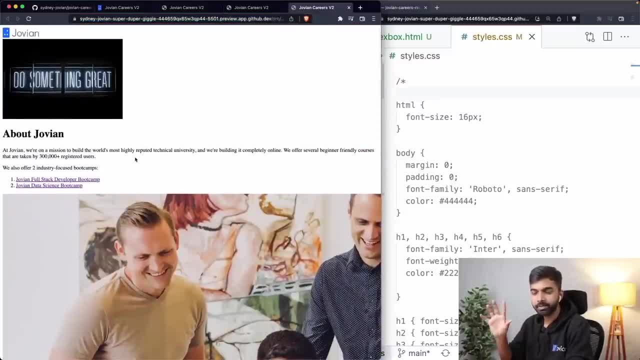 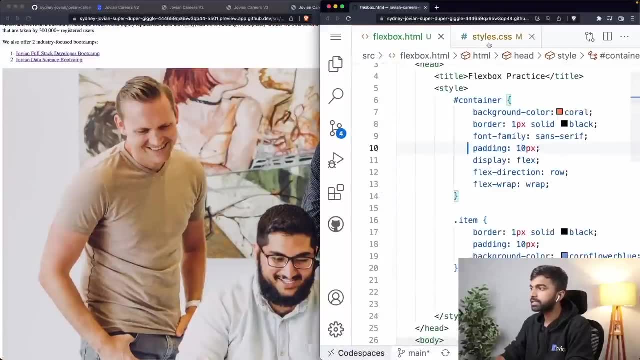 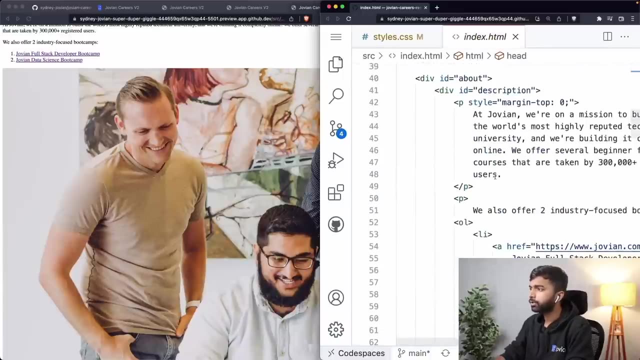 completely gone right. so we have no styles. we're starting from scratch: same content but no css. this one image is looking really big, so i'm just going to give this image a height explicitly in my indexhtml file. i'm going to go into this indexhtml file and i'm going to scroll down. 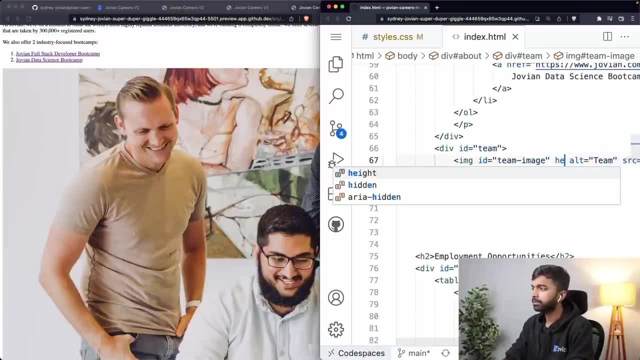 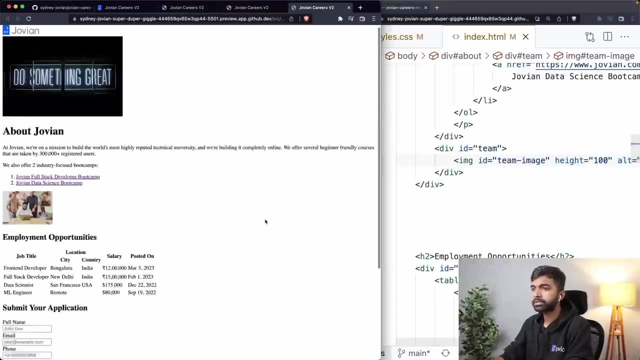 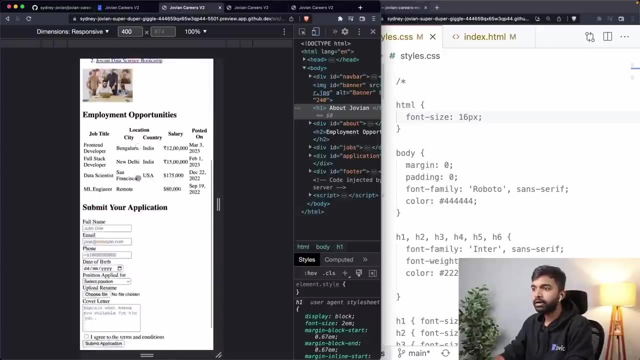 and find this image, the team image, and i'm just going to give it a height of 100 just so that it doesn't mess up the entire page when i'm setting things up. all right, so now we are more or less ready to begin. we have this mobile layout. 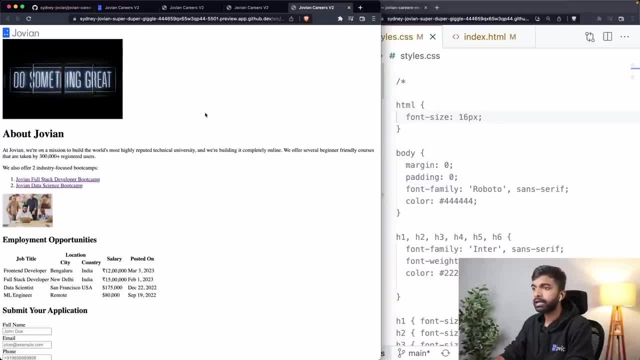 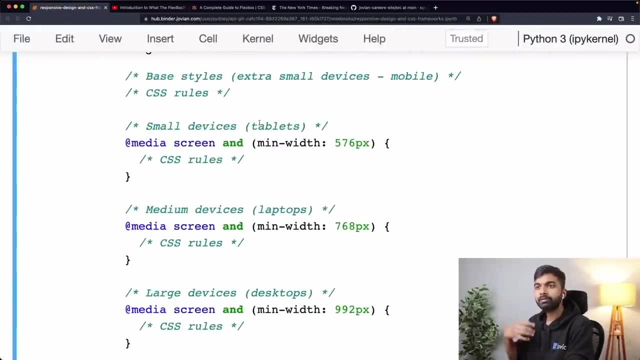 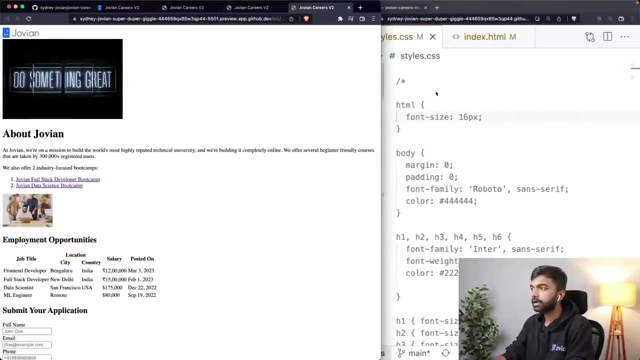 top to bottom content. we have this tablet layout and we have this desktop layout, all right now. let us first just bring in our media queries that we are going to use, for each layout now, the base styles. because we are using a mobile layout, the base styles are just going to be added right at the top without any media query. they are. 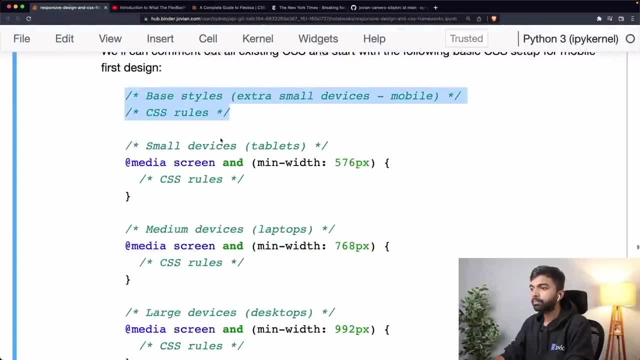 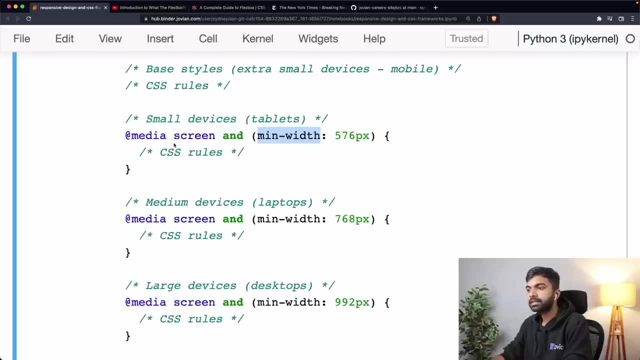 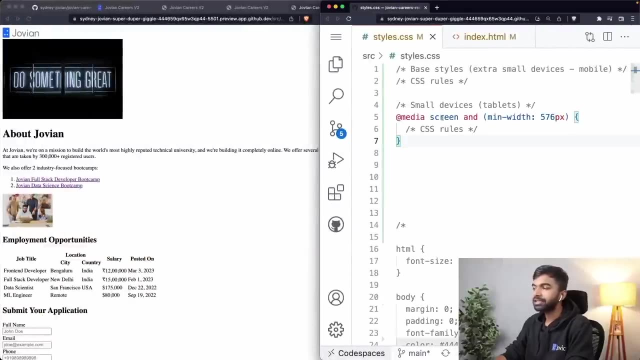 going to apply to all the screens, and then what we're going to do is have this condition called whenever the width of the screen exceeds 576 pixels. then we want a certain set of css rows to apply, and so we are going to then copy over this media query, bring that in, and that is going to. 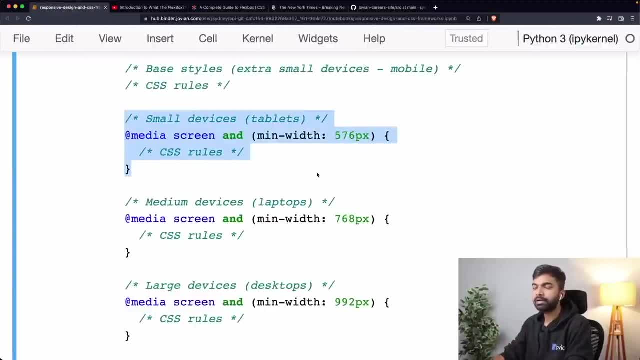 handle tablets. so more than 576 pixels, that is going to handle tablets. notice that it's going to apply about 576 and it's going to continue to apply the same way for all the screens. so that's continue applying unless further overridden in a subsequent query. 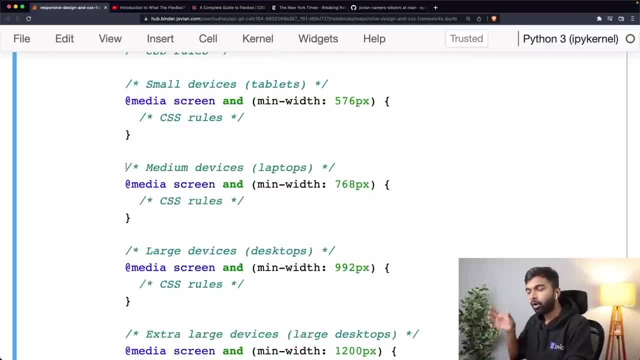 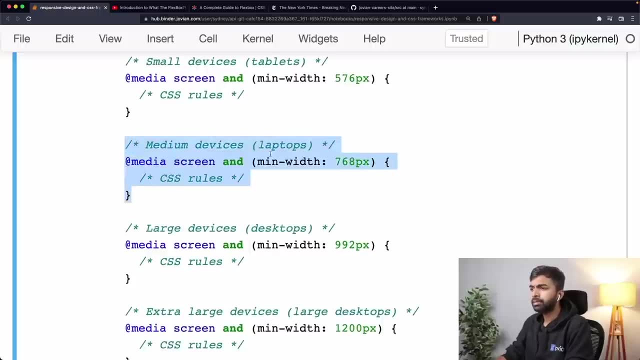 Okay, This way we can avoid a lot of repetition, instead of setting all the properties for each particular possibility. Okay, Then, this is maybe going to be the second media query that we'll use, which is for laptops or maybe desktop screens, proper browsers. 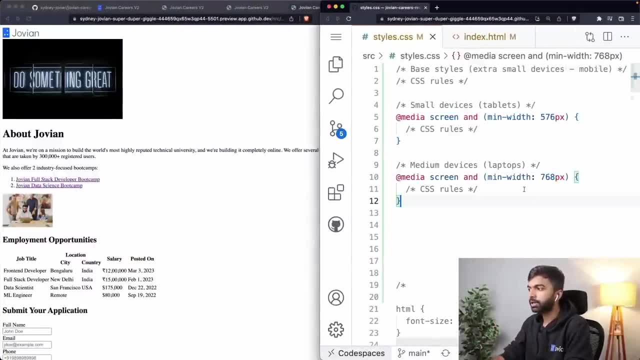 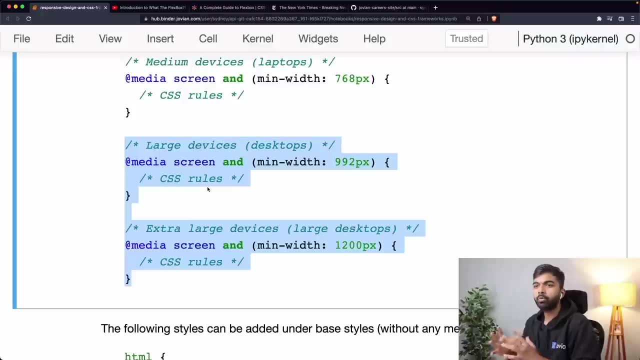 So this is going to be medium devices, or MD, which is going to be above seven, 68 pixels. and then there are also maybe another couple of queries which we may not use, but let's just keep them around: what to do If it's even bigger, if it's bigger than 900 pixels and if it's 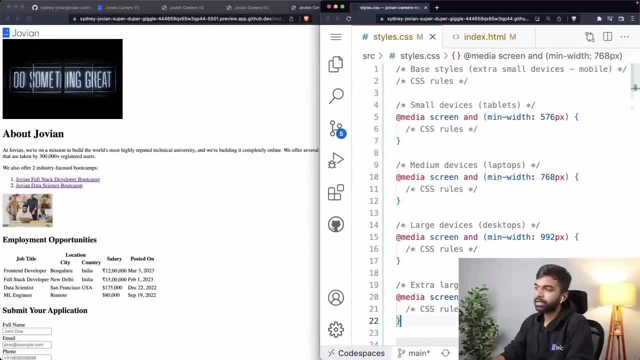 even bigger than 1200 pixels. again, we don't have to use these, but if you want, we can maybe increase the font size, of base size, a little bit, or something like that. All right, So now our basic setup is ready. 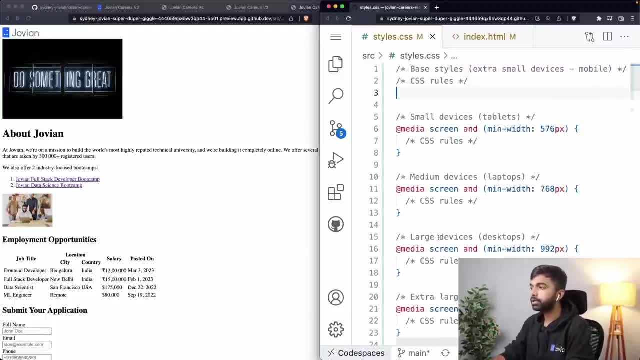 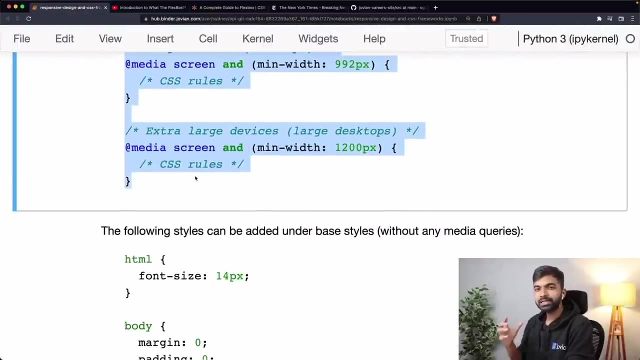 We have this: we have like basic CSS rules that are going to come here. You're going to then add device specific or Um, progressively enhance our design to tablet and desktop. Okay, Looks good, Looks good. The next thing to do is to just set up copy over some of the basic. 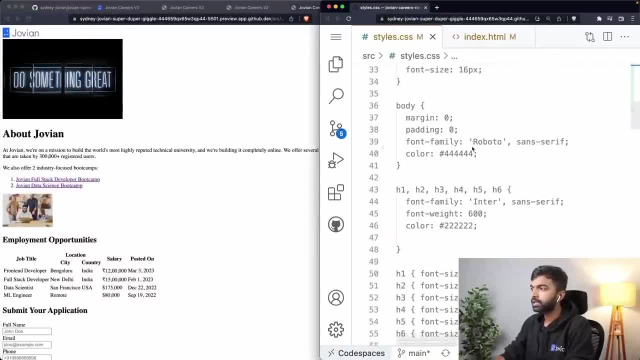 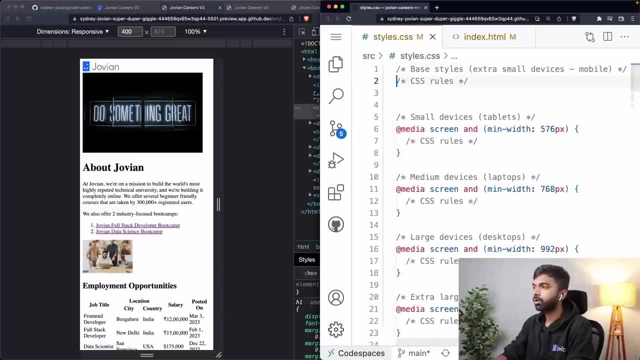 styles, without any media queries. I'm going to first come in here and I'm going to say that the font size, the base font size on mobile, is going to be not 16 pixels but 14 pixels. I just want the font to be slight. 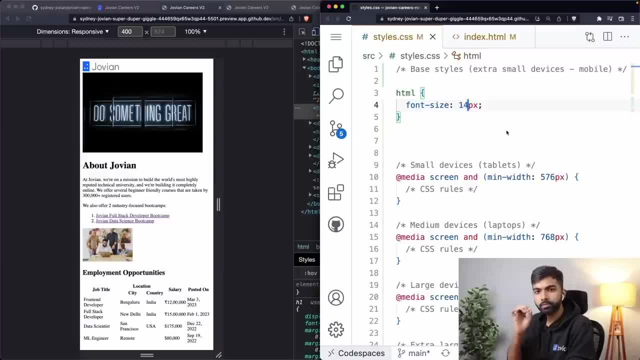 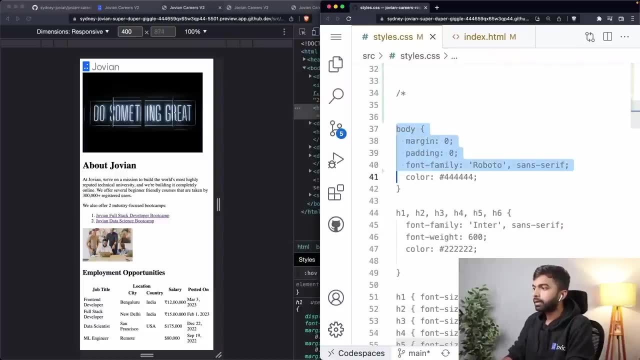 Slightly smaller. I don't want it to be too big on mobile because otherwise there may not be enough content on the screen to be readable. So let me keep that And then let me come in here into body and let us come in and let us. 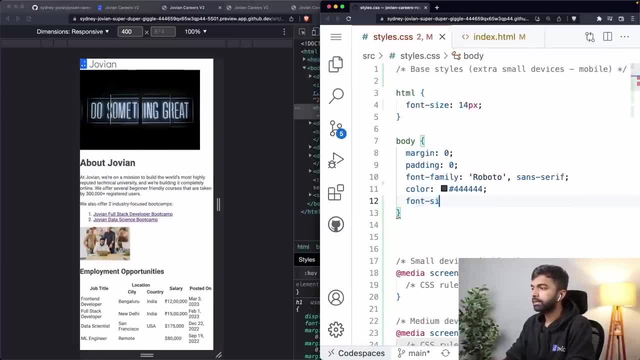 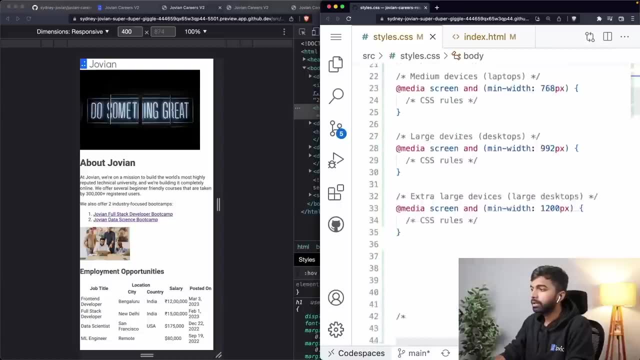 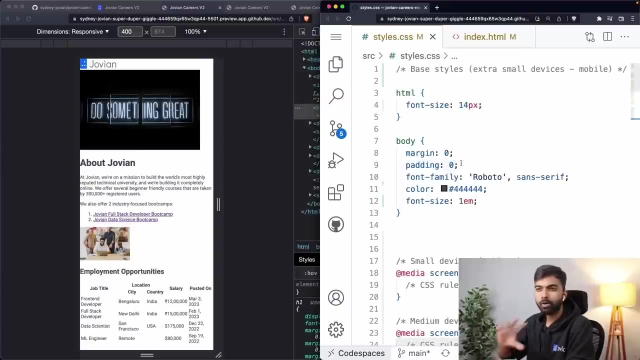 set the font size for the body to one EM, one M. that is going to be the font size for the body. Then let me come in and let me set uh apart from the font Size for the body. We've also set here that we've removed the margin padding. 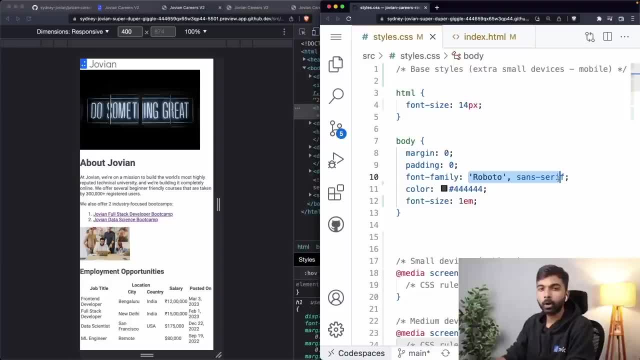 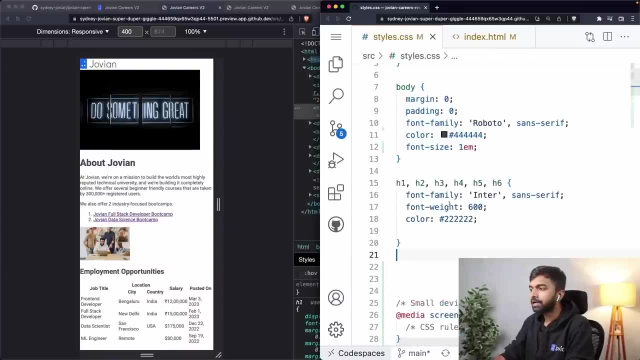 All of this needs to go for mobile as well. You've said the font family to Roboto and sans serif, and we've said the body text color to four, four, four, four, four, four. Okay, great, Let us now set the font family and the font weight for our headers. 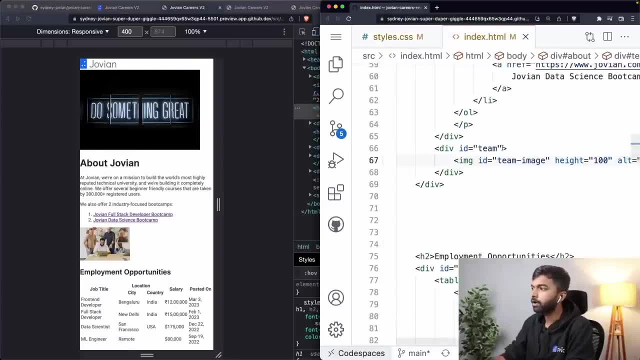 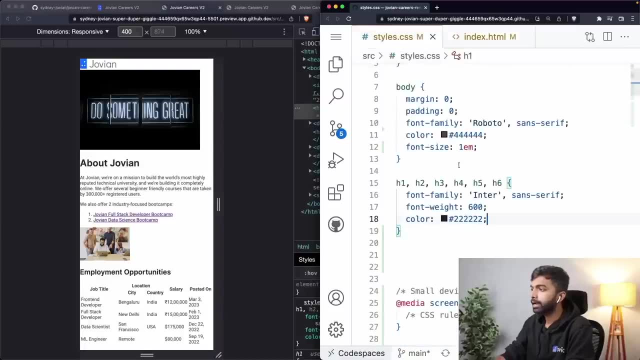 So we want the inter font family to be used And remember these font families have been included using these link tags. You can see here that we've included the intern and the Roboto font family And they are various weights. All of this is common. 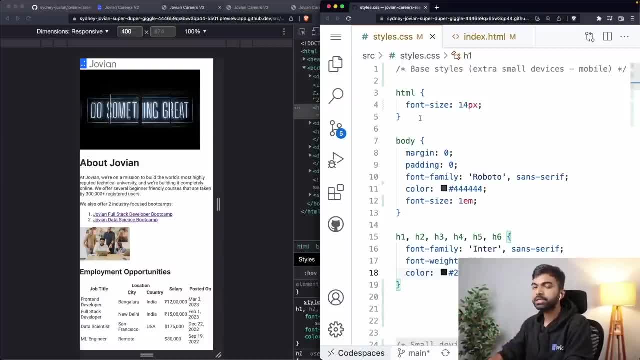 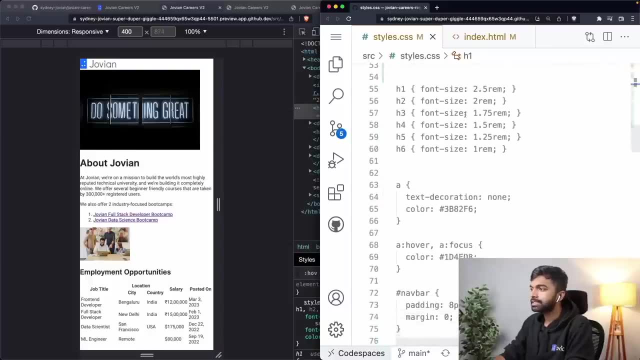 All of this is going to be present on mobile, tablet, desktop. That's why we're just putting it completely outside. Okay, So that's fine too. Then let us go in and let us set the font sizes for each header. So remember we are using these ramps. 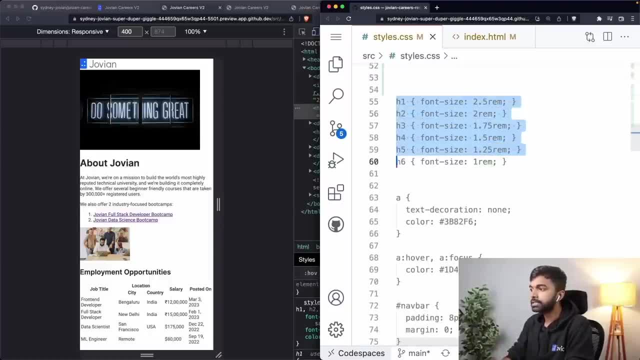 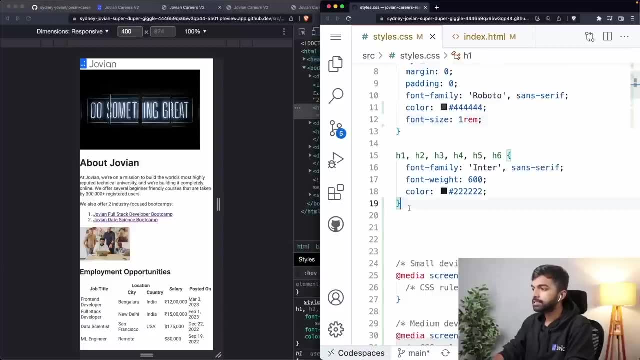 We're using REMs or relative measurements, or the headers, so that on mobile screens they are going to be multiples of: or let's set this to one ramp on mobile screens. Uh, they're going to be Multiples of 14 on mobile screen. 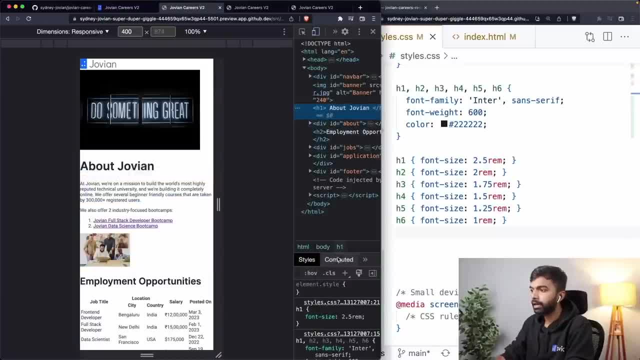 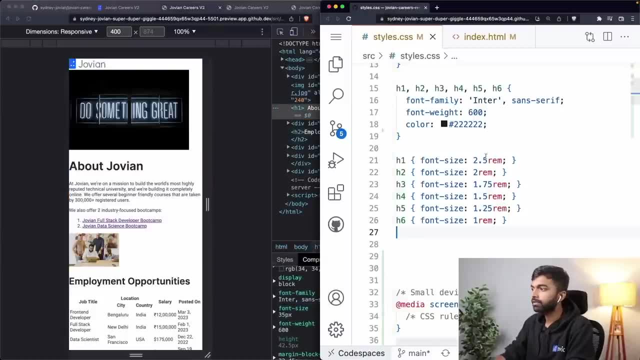 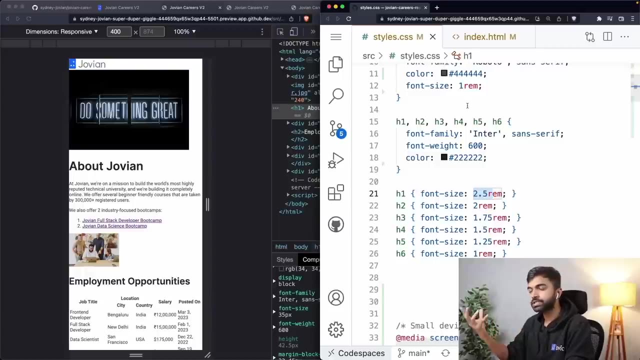 You can verify here. If I go into peck and I check it's computed font size, you can see that it's 35 pixels. 35 is 2.5 times 14.. Okay, But as we go on to bigger screens, we're going to set the base font size to 16 pixels. 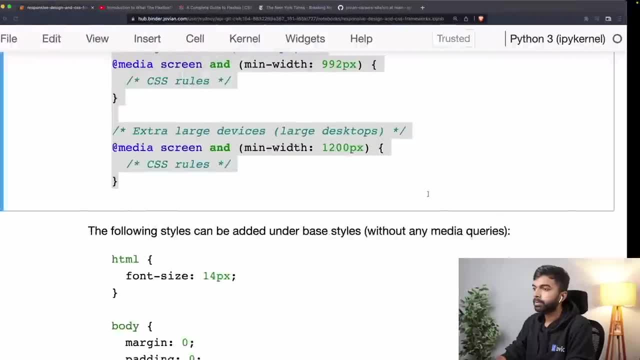 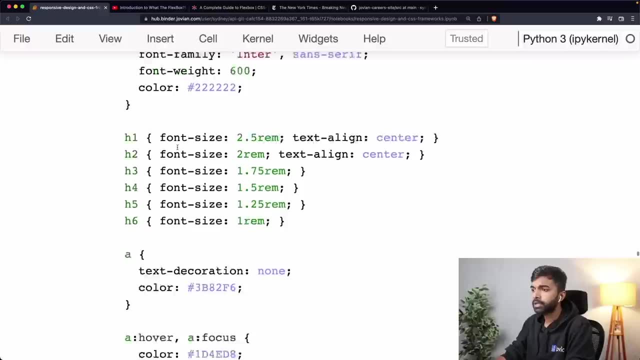 And so the header size is going to increase as well. Okay, What else? Yeah, I think that's what we've added. So you added HTML. Yeah, Yeah, HTML, um body H1, H2, and let's add a couple more. 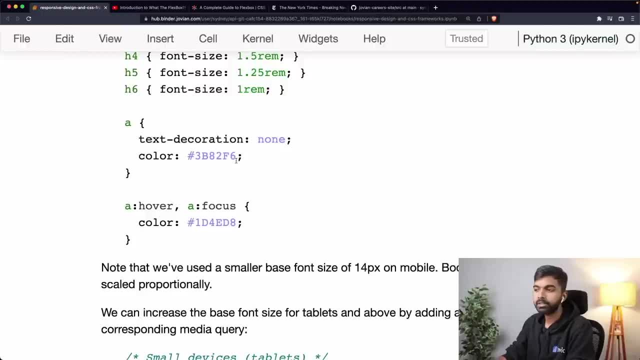 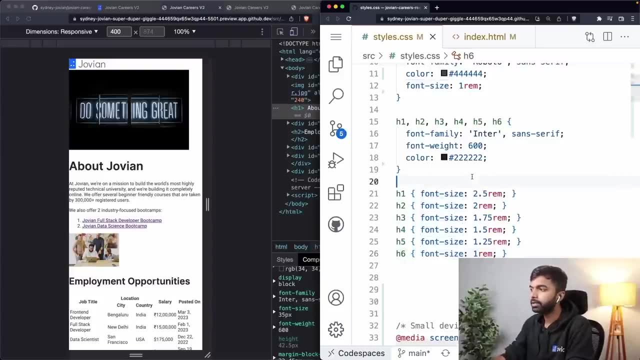 Let's add the text color and let's add the- uh, the style for the links. right now You can see that links are underlined. I don't want that And I want links to be my brand brand blue color. So that's where I'm going to go in and grab this decoration text. 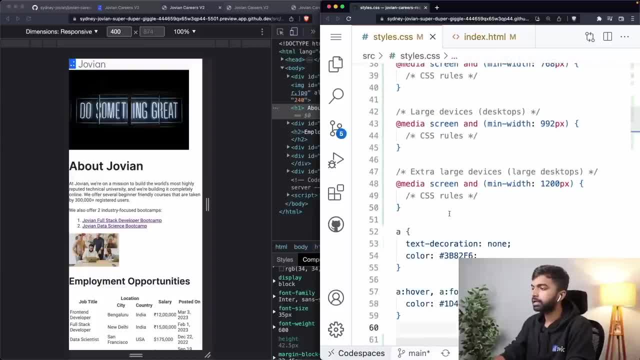 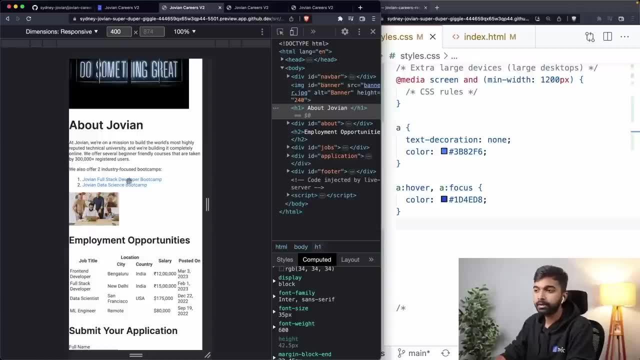 decoration or the links. Let me put that in here as well. Okay, So, yeah. So now you can see that if I reload the page, I would links, have the desired color. they don't have an underline and on clicking our links, 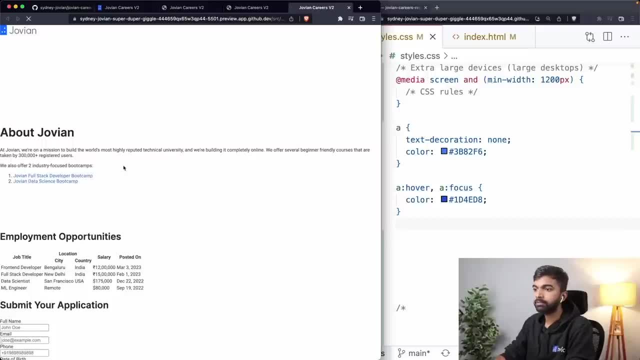 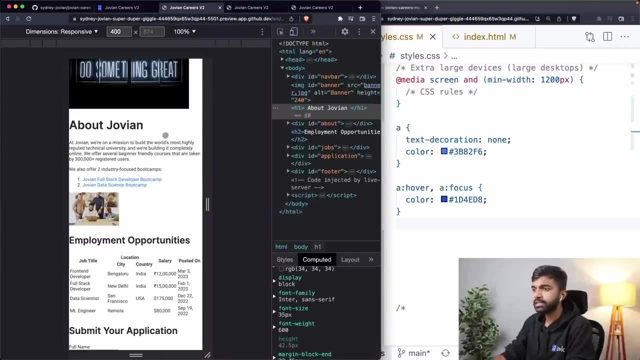 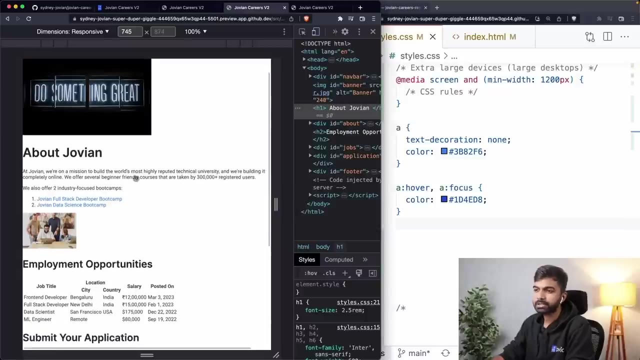 have the desired dark color, or, or, or our links have the desired dark color. All right, So now this is looking good. So far, we have said the base styles. let me just reload this page. Yeah, we have said the base styles. now we, and of course it just spreads. 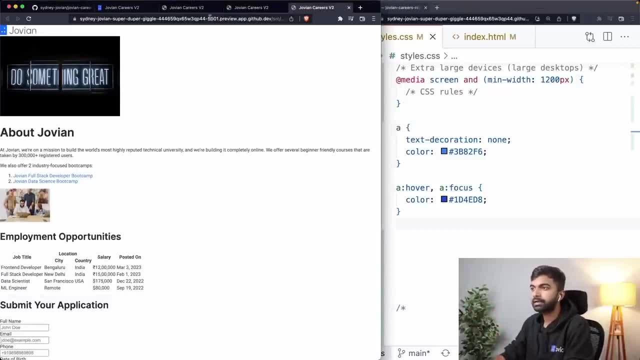 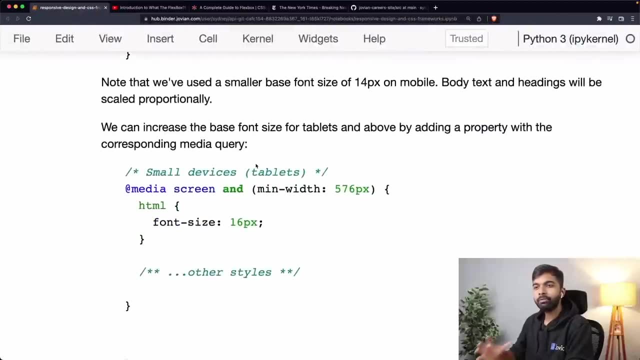 out on tablet as well, So there's nothing that really is changing across the different layouts. The first change that I want to use is when we get to a tablet style. I want to use a slightly bigger font size for the body. Okay. 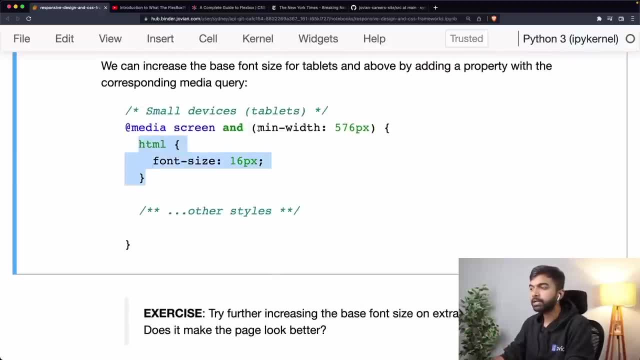 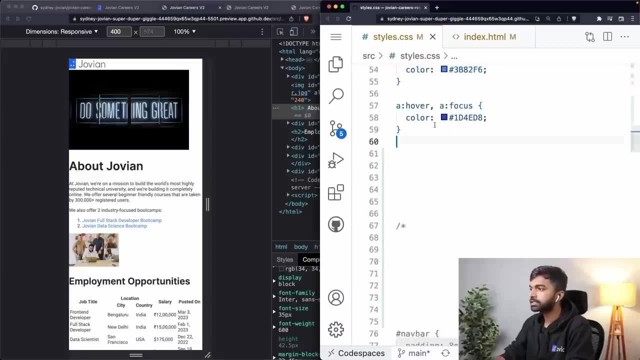 So within the media query where we hit a min width of 576, I want to use a slightly bigger font size. I'm just going to come in here and I am just going to use a bigger font size here. So I'll just come into the first media query, which is over here. 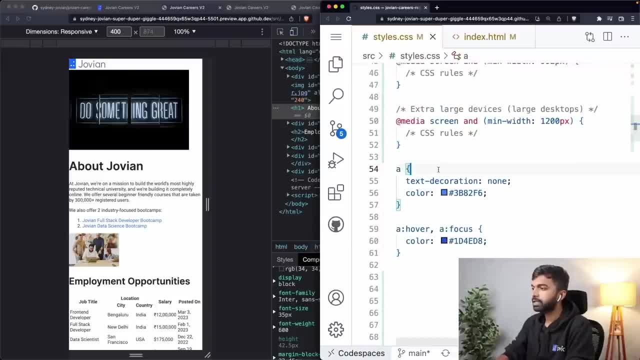 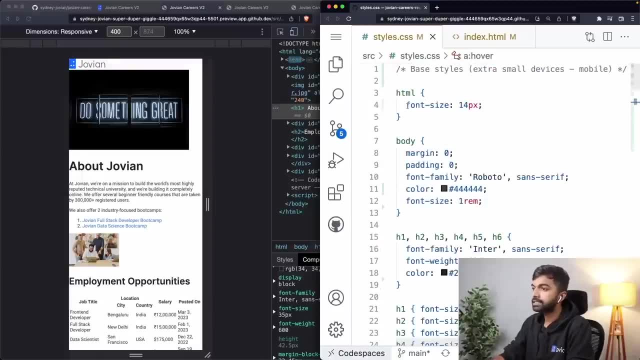 And I'm going to put the font size of 16 pixels. Let's move these up. Let's keep it- All the base styles- right at the top so that things are well organized. So these are the base styles. The base font size is 14 pixels. 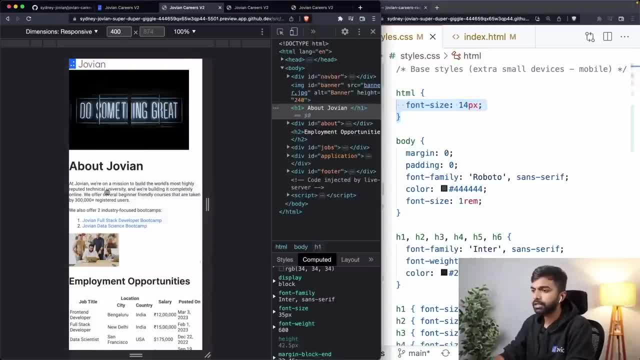 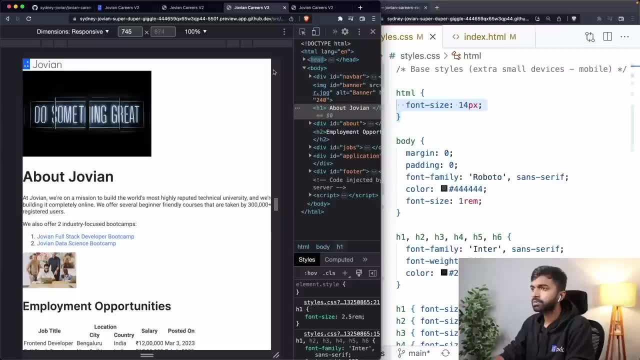 No change here. You can see that the base font size is 14 and actually go in and check somewhere that the font size is 14.. But as soon as we hit a bigger font size, as soon as you hit a bigger screen, as 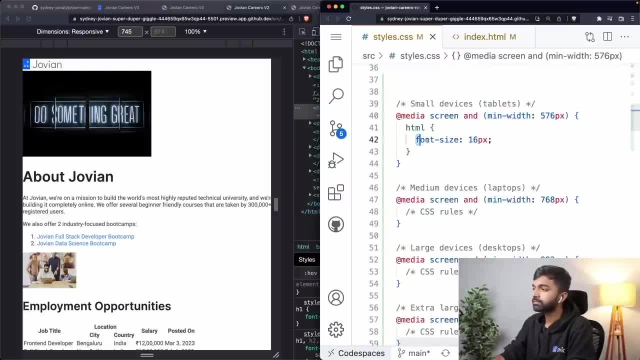 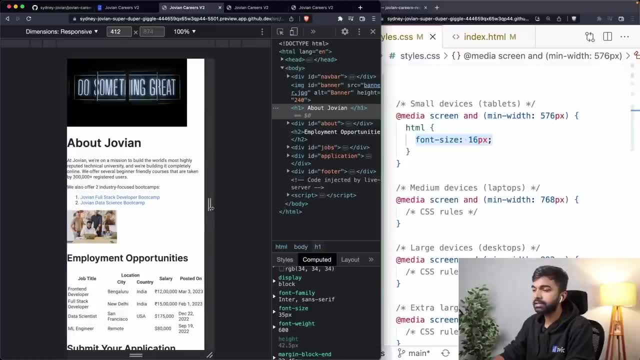 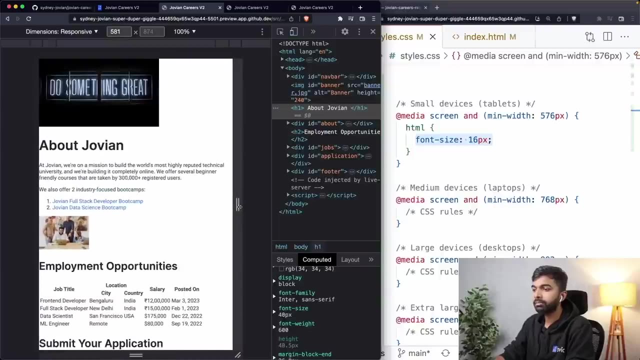 soon as we hit a min width of 576 pixels, the base font size changes to 16 pixels. You can actually Observe this change in the font size by just dragging this 576, the text should become slightly bigger. You see here that the text became slightly bigger and not just the text, because we are 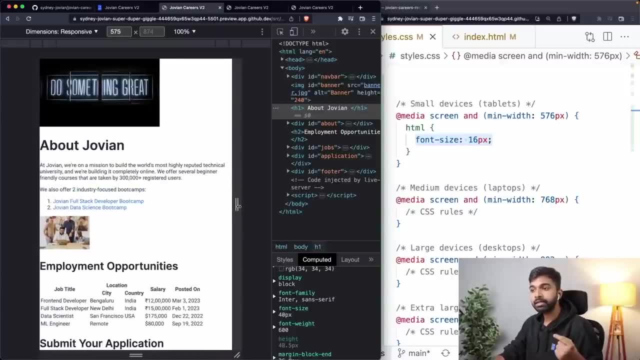 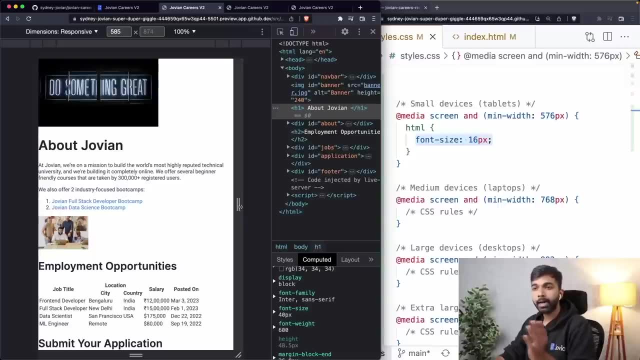 using the rems to set the size of the headings, You can see that the headings have become slightly bigger as well. So this is one change that you will often see that from mobile to tablet, or maybe from tablet to desktop, there will be a slight change in the font size. 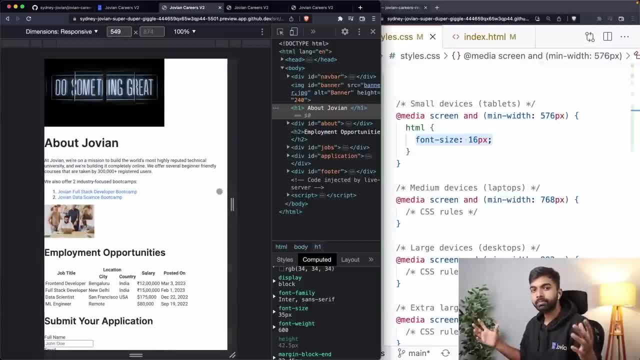 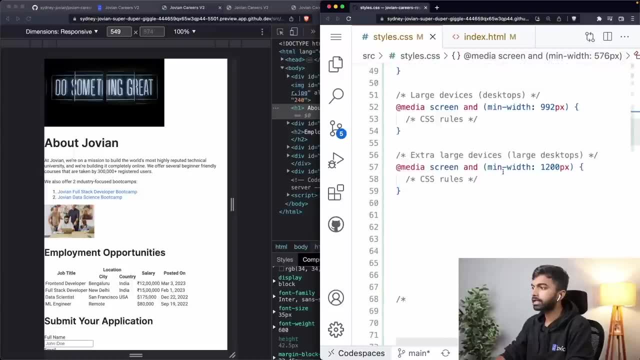 Of course you can go ahead And maybe change. Let's say, you get a very big desktop, a very big screen. You can use the base font size of 20 PX. Let me just come in here and let me just show you what that would look like as well. 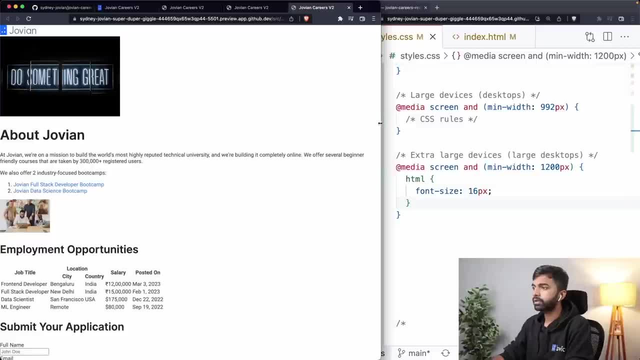 Even ever we hit 1200 pixels. I want to use 20 PX, So so far at 16, at some point it should become 20.. Okay, Maybe I'm still not hitting 200 pixels. Let's try that at maybe nine, 92 pixels. 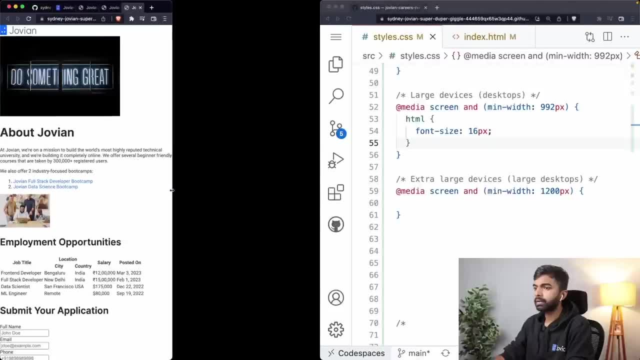 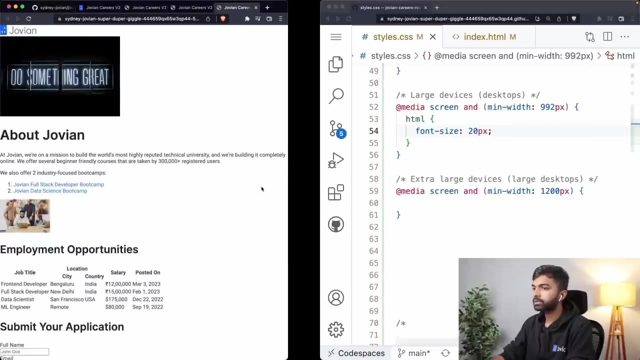 Yeah, you can see that it's small here. So this is the tablet layout, and at nine, 92 pixels it becomes bigger, right, And then, of course, on mobile it is even smaller. So you have all those. well, actually it said that to 20,, but nine, 92 pixels. 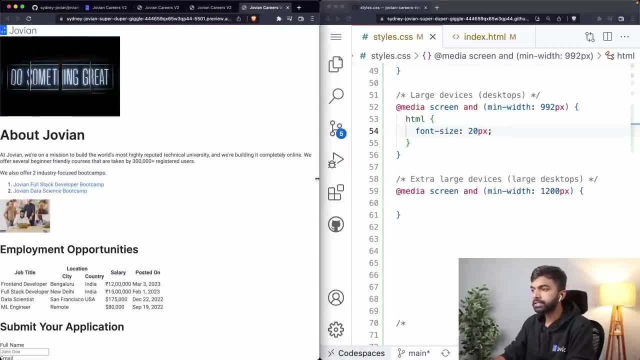 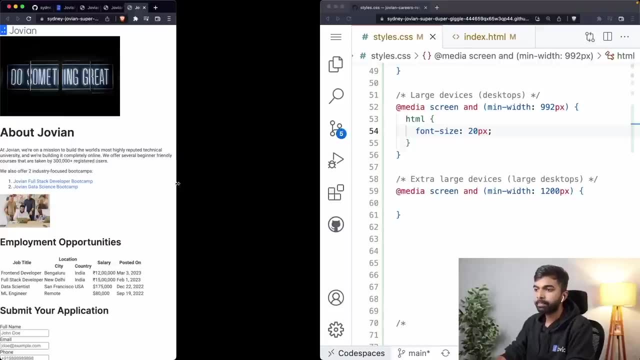 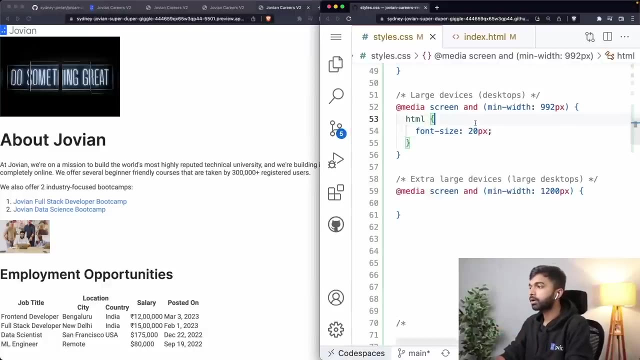 it should become bigger. Yeah, You can see that just around nine, 92 pixels, it starts to become even bigger, Right? So I know this is mobile and this is Tablet and this is the large desktop. Okay, These are all the variations that you can check. 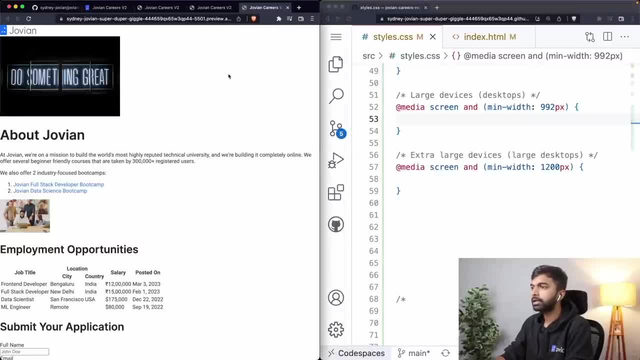 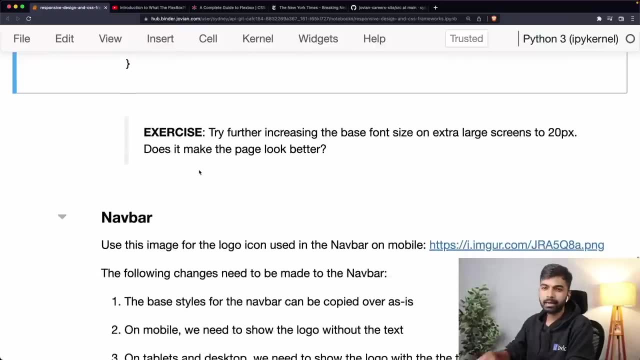 And sometimes you just have to inspect things visually and figure out if you're getting what you're going for. Okay, All right. So now we've changed the base text size and I encourage you to maybe change some other base styles, maybe change base heading sizes as well, and see what happens. 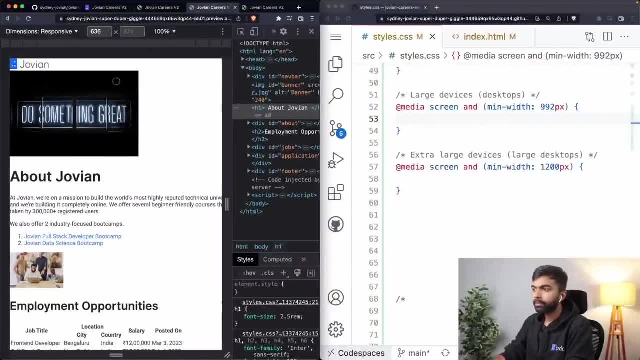 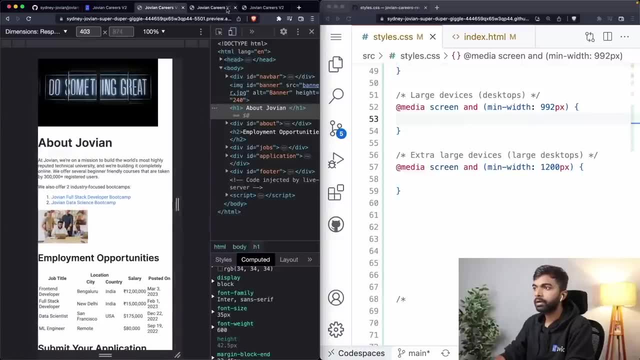 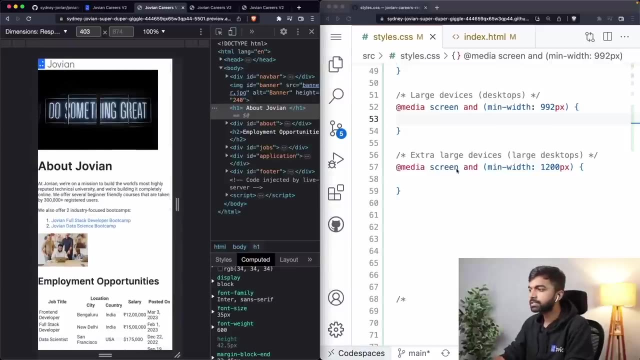 Now the next thing we'll do is fix the nav bar, Okay. So first let us Implement the nav bar from for mobile, Let's bring this back to about 400 and let us go check the nav bar. Okay, So now we need to bring in the basic nav bar styles first. 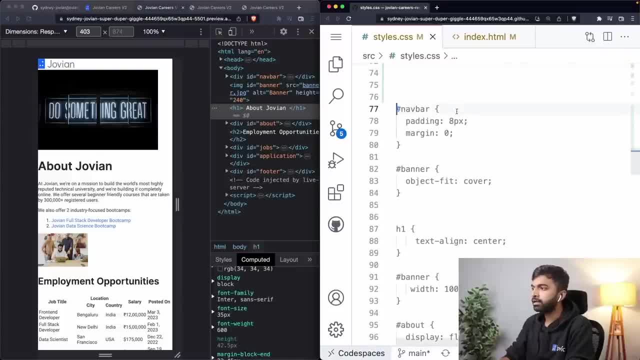 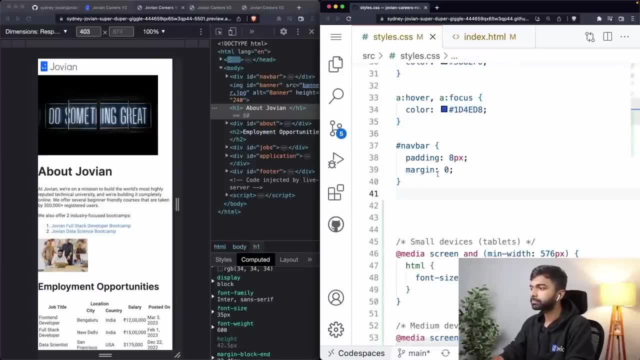 So let's bring that in here. The nav bar has a padding of eight pixels and a margin of zero pixels, So let's just bring that in. I think we can keep that. I don't think we need to change that. I'm just going to bring it all the way at the top. 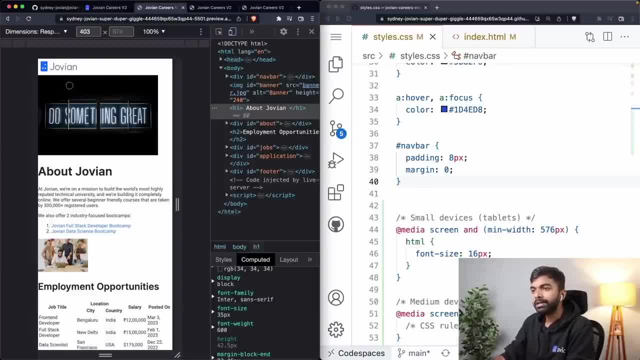 You can see that our nav bar is starting to look fine. Now, one thing I want to do in My nav bar is not use this entire logo, but maybe use a smaller version of the logo that contains just this icon and not the text. 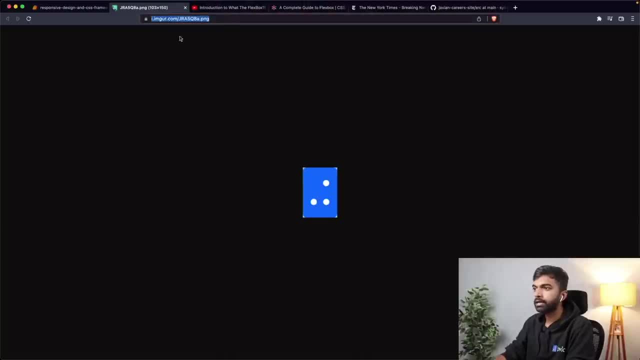 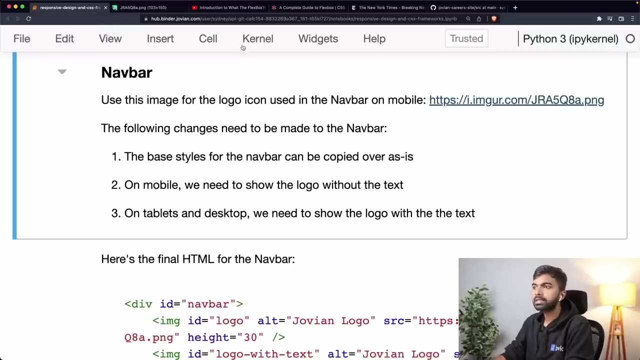 And for that I have already put up this icon online. so I can just use this link, or I can download it, drag it within my code space and add it to my repository. Both options are available. Let me do one thing. Let me just add this icon into my code as well. 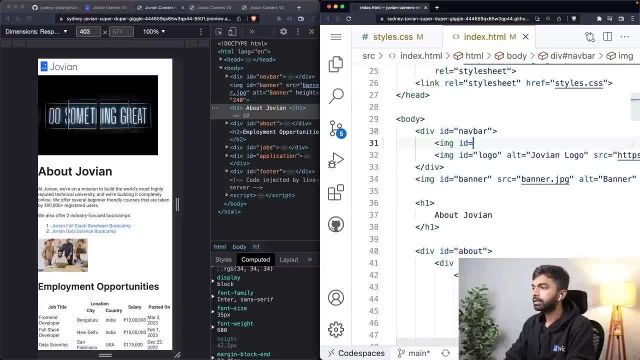 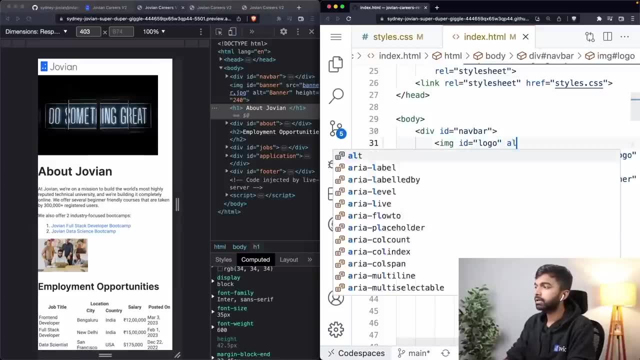 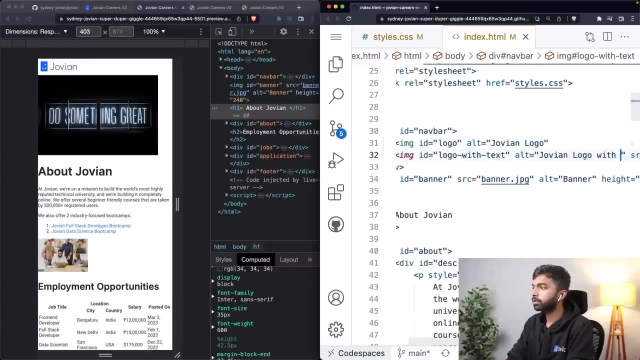 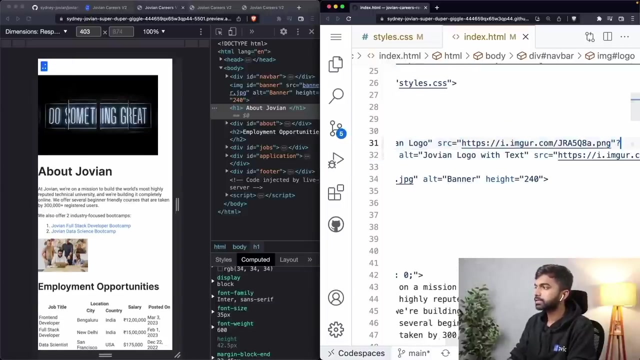 So let me just go. IMG ID logo. I'm going to change the icon I can with the text to logo with text. then all equals login logo. I'm going to change the old of the existing icon to join logo with text. Let's specify an SRC and let us close it. 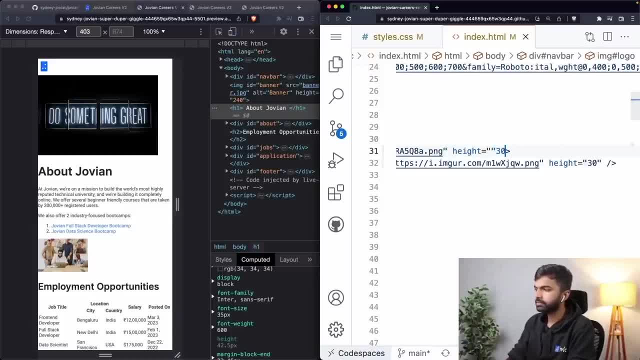 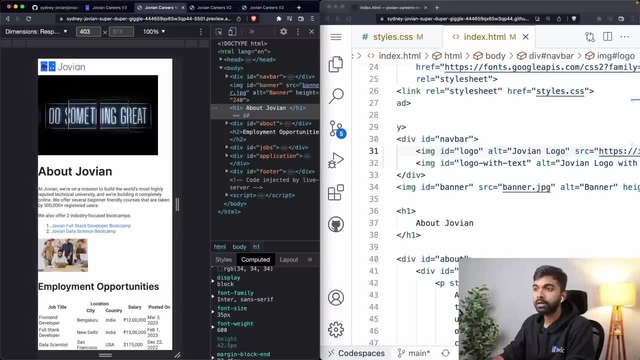 And I think we have a height 30 as well, So let us set a height equals 30 as well. I don't think we need to change the height particularly. Okay, Now we have both these images. We have the icon image and then we have this logo along with the text. 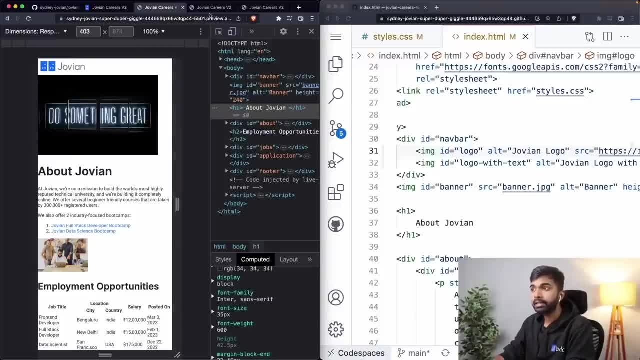 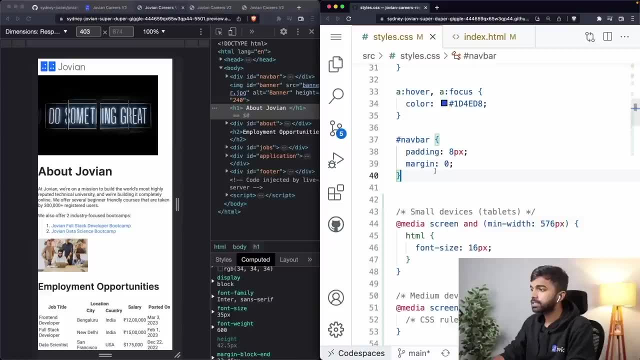 Now we want to show one of these on mobile and then on tablets. I think we have enough space that we can show the entire logo with the text, So here is how we can achieve this. First, we want to hide this icon. You want to hide this icon? 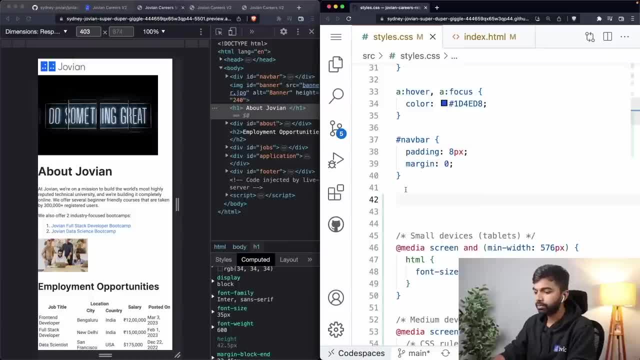 We want to hide the logo with the text on mobile. So by default I'm going to keep it hidden. And the way to keep it hidden is let me just select logo with text. So I'm selecting it With the ID And let me just set display: none. 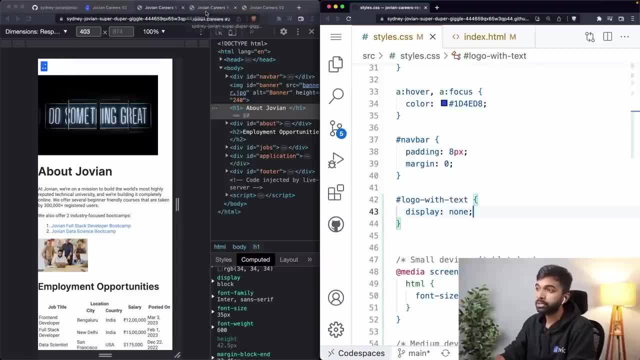 Then it's gone. The logo with the text is gone. It's gone not just on mobile, but it's gone on tablet and it's gone on. It's gone on desktop as well. Now let me make this logo text visible on tablet. 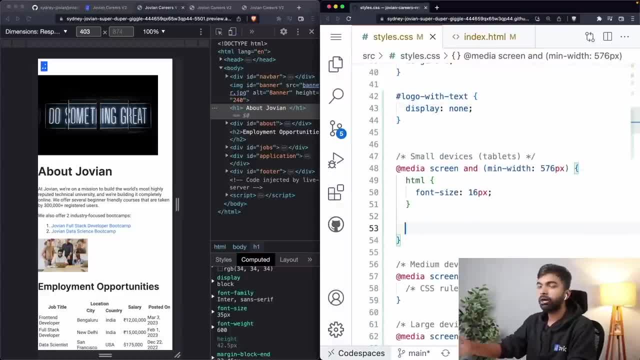 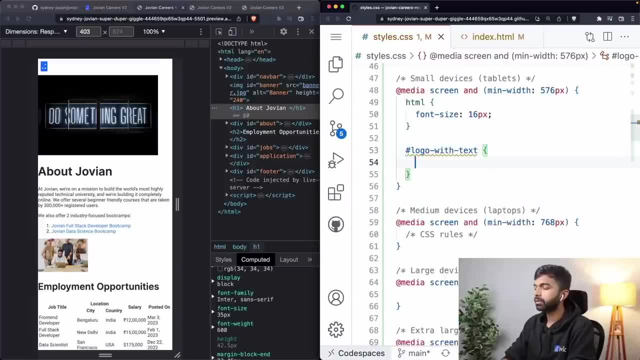 So I am just going to go into the tablet style which is above 576 pixels. on min width of 576 pixels. I'm going to say logo with text Display. I can just say I believe I can do lock, which is the default. 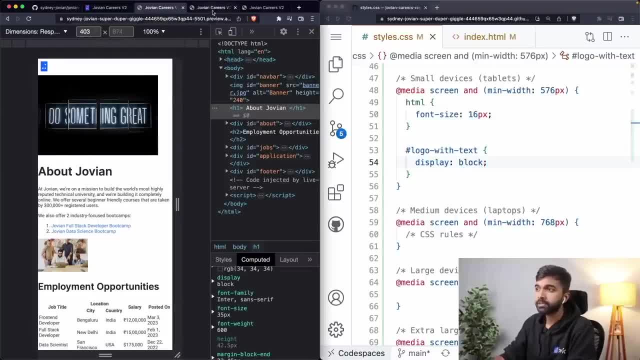 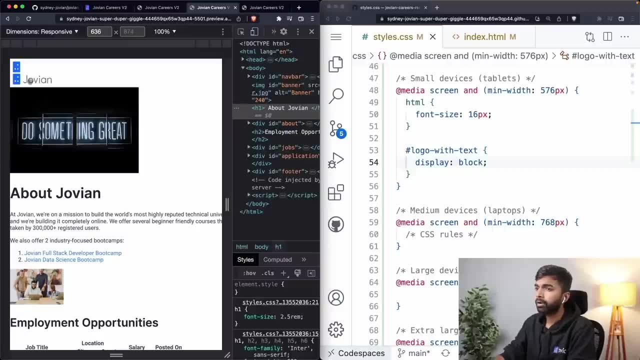 Now, it doesn't show up on mobile which is under 576 pixels, but it does show up on. Yeah, it does show up here on tablet and it does show up here on desktop as well. Okay, But of course, we also need to hide the logo. 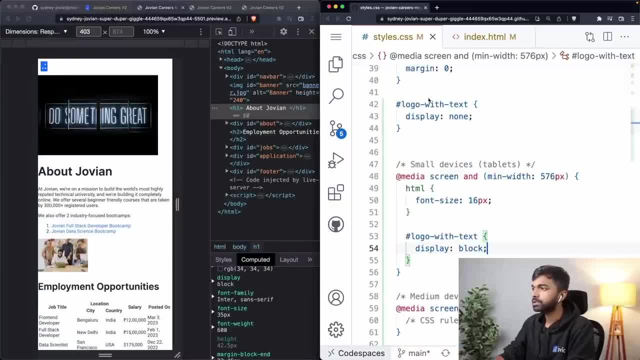 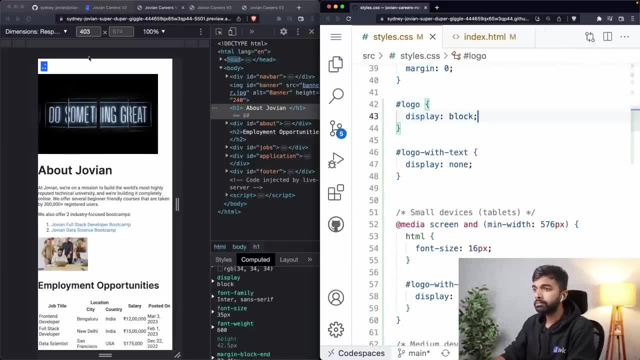 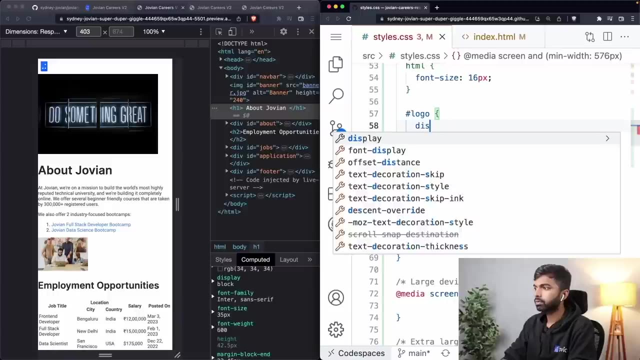 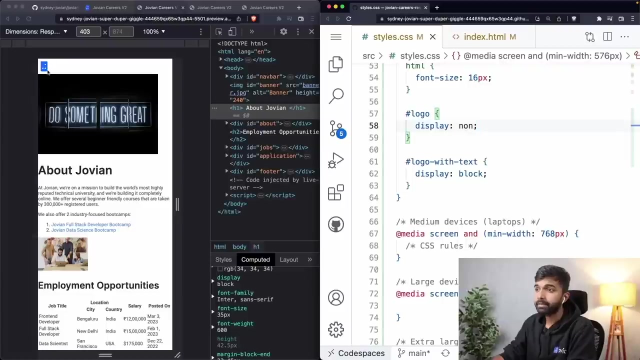 We need to hide this logo I. So I can just also say over here: logo display block on mobile. and I can just say: logo display none on tablets. Okay, So on mobile I have the logo, only the icon on tablets. 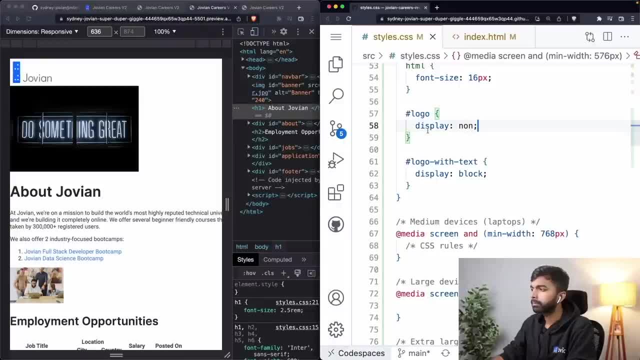 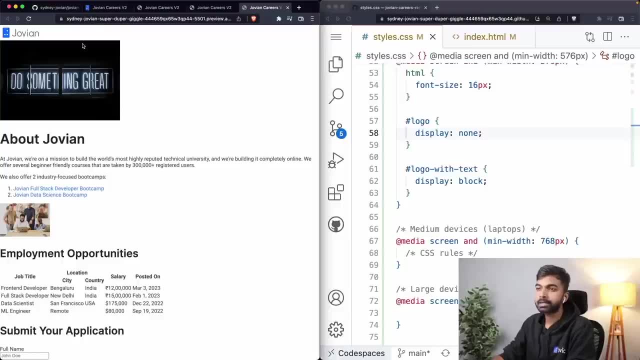 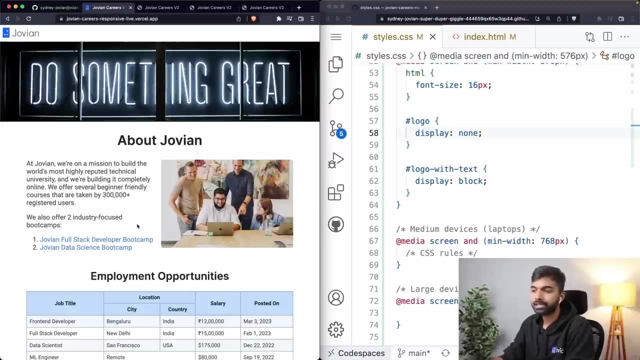 I have the logo with the text and also on bigger screens, I have the logo with the text, but that takes care of the Napa. That is a change that I'm going for. That is a change that we have on our website as well. 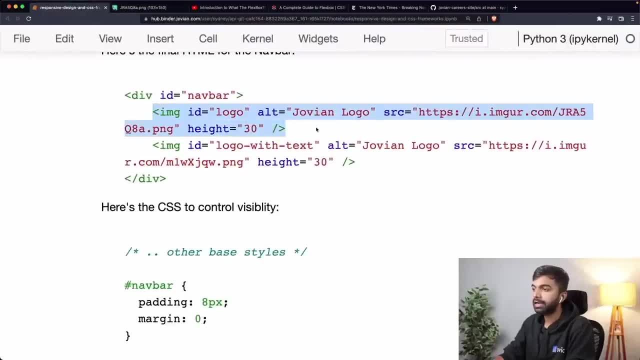 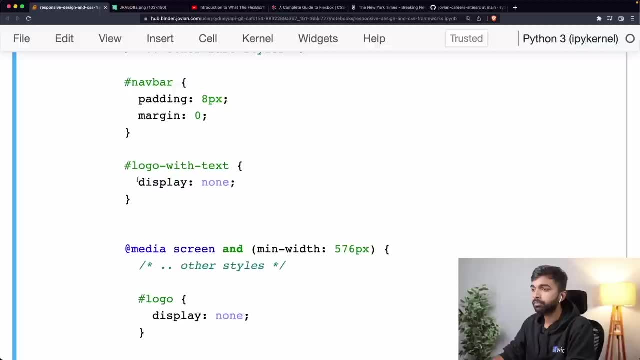 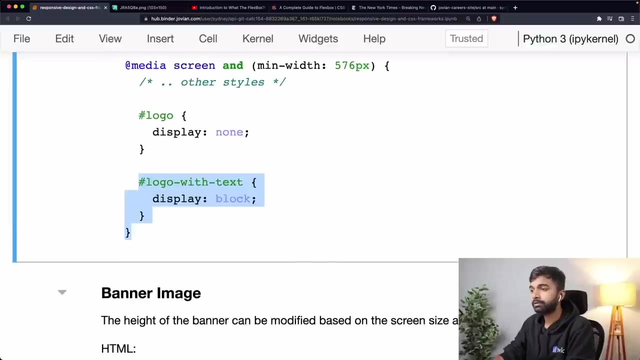 All right. So the Napa is taken care of and the only change we made is added this second image and we have added the base style where we are putting the padding in the margin And we have put The logo with text as display none. and we are going it on tablets and desktops and we are not showing it on, we're not showing the icon alone on tablets, and notice that once we apply it for tablets- because this is this- only has a min width criteria, not max width- it's going to apply it all bigger sizes. 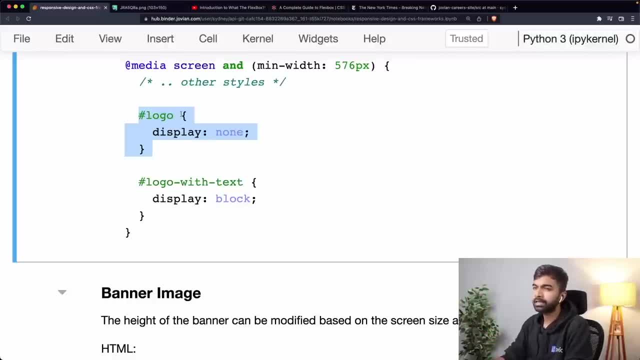 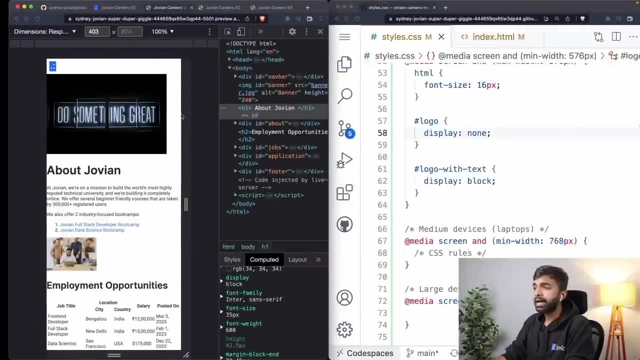 If I want, I can then go in and change it at a bigger size as well. Otherwise I can leave it as a so mobile. first progressive enhancement, section by section. Okay, Let's fix the banner Image. So the there are a couple of issues with the banner image. 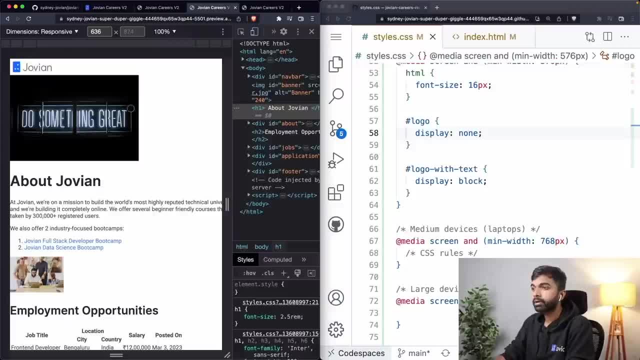 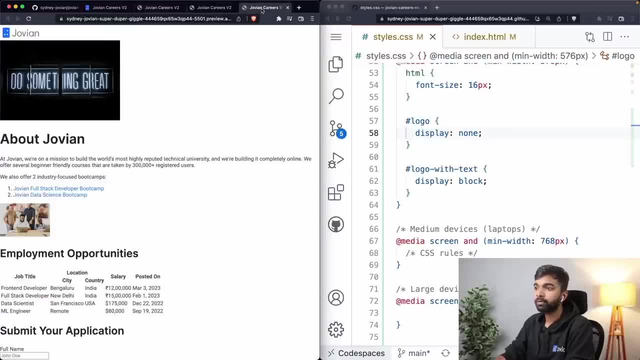 One is that it's not taking up the entire width of the page And second is that I might need to limit the height of the banner image or each of the weights that I'm working with. Okay, And I want to do that, Let me just do that. 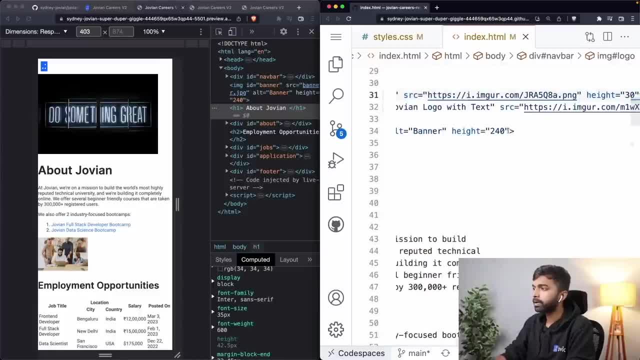 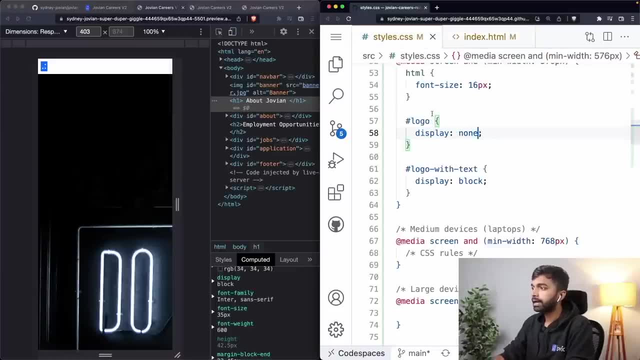 So the first thing I'll do is go into the banner image. It looks like it has a height. Let me remove the default height so that I can change its height based on the specific breakpoints, And let me come in here and let me just 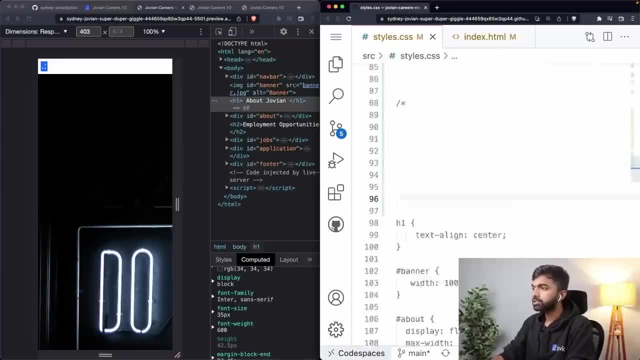 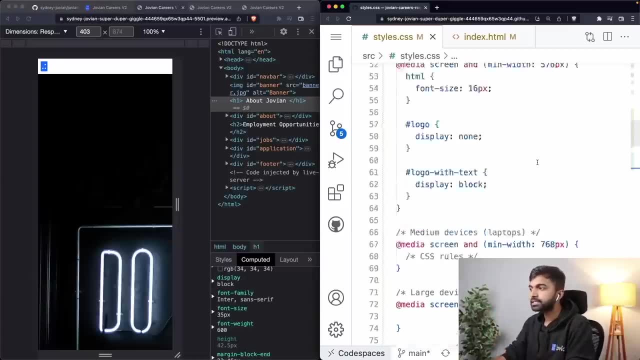 Copy over some of the content that I already have for the banner, So we have object fit cover. This is to make sure that, depending on what width or height we have, it automatically fills the space, the available space. Okay, And here's the first thing I'm going to do. 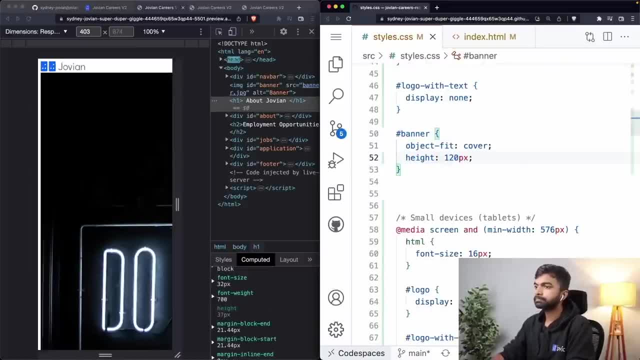 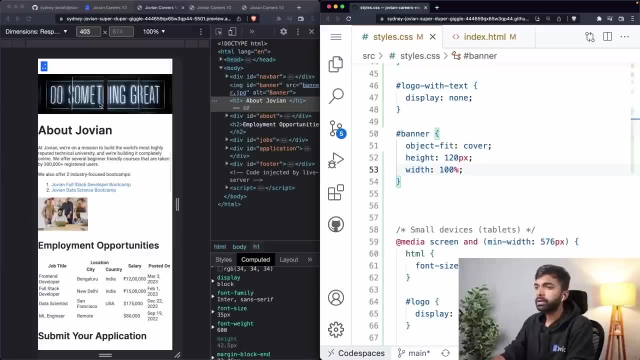 I am going to first give it a height of just one, 20 pixels- the banner image- and I'm going to give it a weight of a hundred percent. Okay, I think that looks good, So maybe one one, 50 pixels. 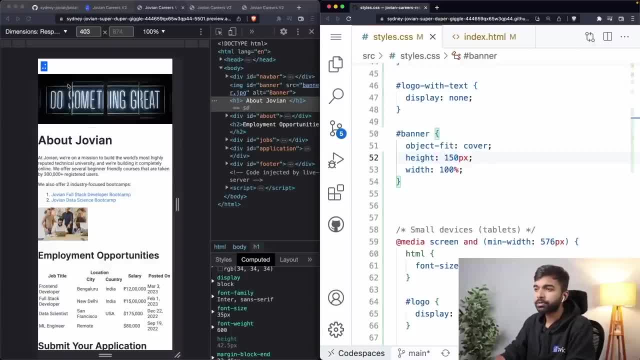 Let's see. Yeah, that looks good. So now on mobile, this is what it's going to look like. It's going to take a one, 50 pixels, and it's going to take up the entire width of the page and it is going to cover. 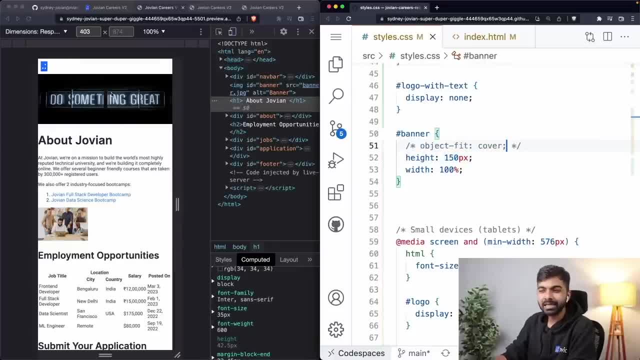 So if we did not have object fit cover, you can see that it stretches the image, which is not good. I don't want to stretch the image, especially if these are faces of people. Always use object fit cover or sometimes you might need to use object fit contain. 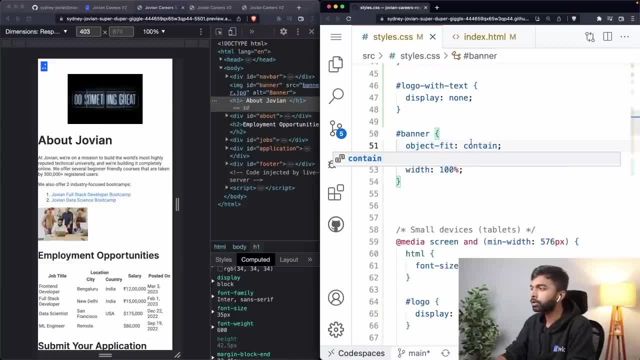 If you want to, if you want the entire image to fit inside. it's not what we want here. You want to cover, So let me just put a quick cover. Okay, Okay, Okay, Okay, Okay, Okay Okay. 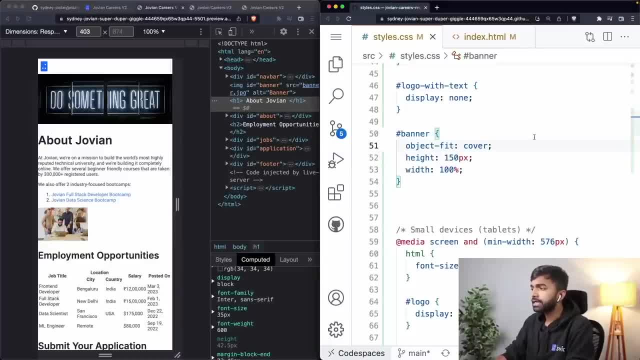 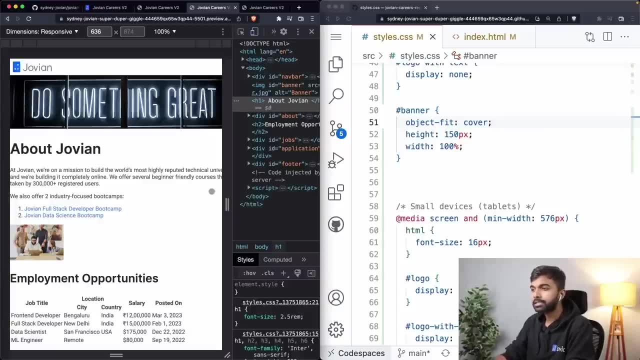 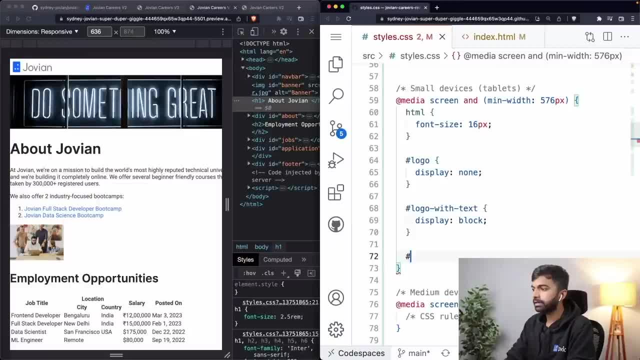 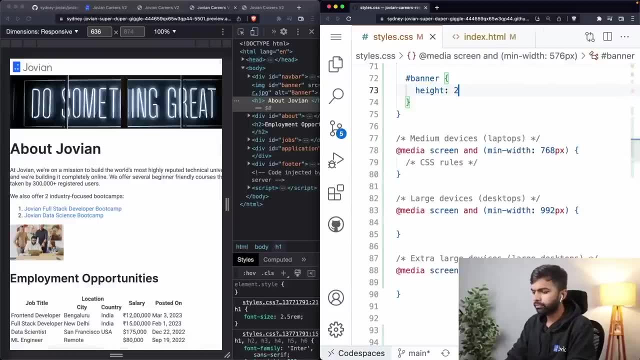 So on. maybe on tablets I can increase its height a little bit, So I can say banner. I can give it a height of two, 20 pixels. How about that? I think that looks good. Maybe even 200 pixels should do it. 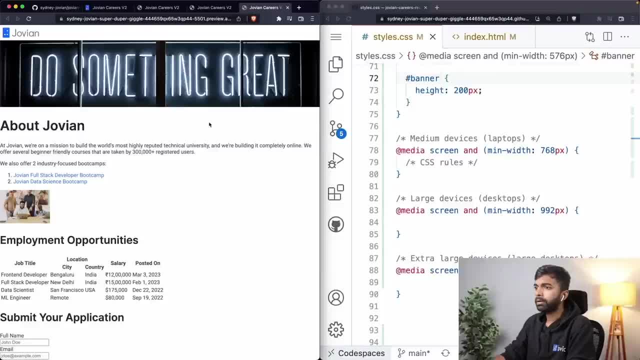 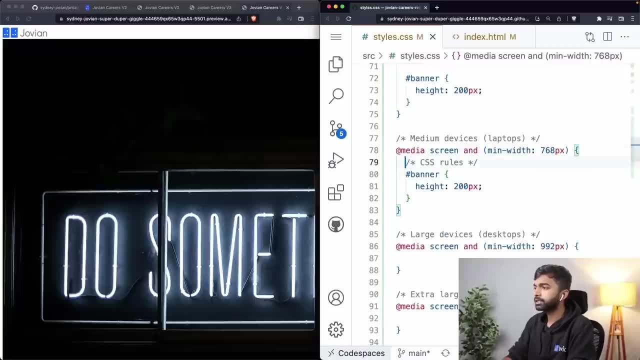 I think that's good. And then, here again, it seems to be getting cropped a little bit so I can come in. and I can come in into the next design, And this is the first time I'm touching the desktop design. so far we've just been updating. 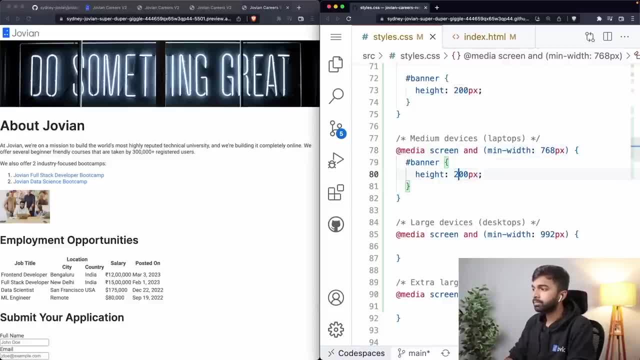 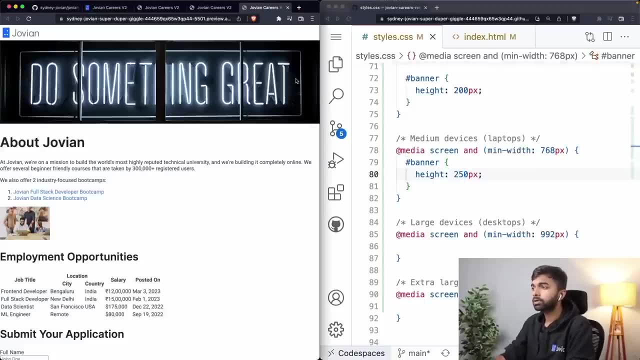 for tablet and that has carried over to desktop. So here I can maybe give it a height of 240 pixels, maybe even 250 pixels. This is now looking good. Okay, I should probably verify that the scales properly. Okay, Maybe I need to give it a little higher. 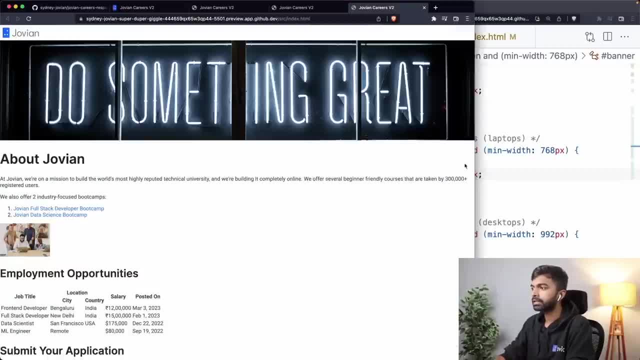 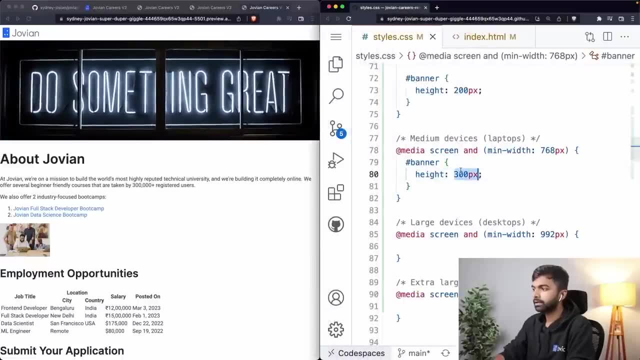 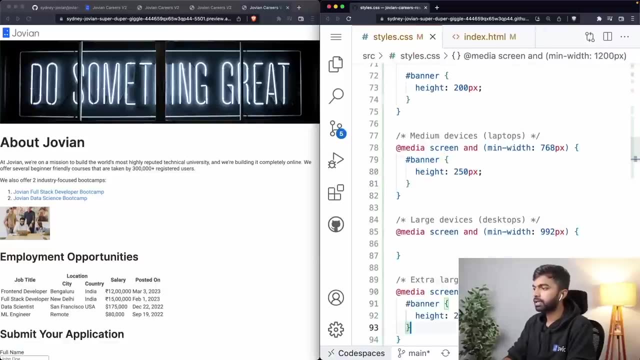 Maybe let's go 300 pixels. Yeah, I think that looks good so far at this as well. but if I wanted, I could even just do something like two 50 pixels here and then on even bigger screens. I could just go in and I could just make that three 20 pixels at some point is going to become even. 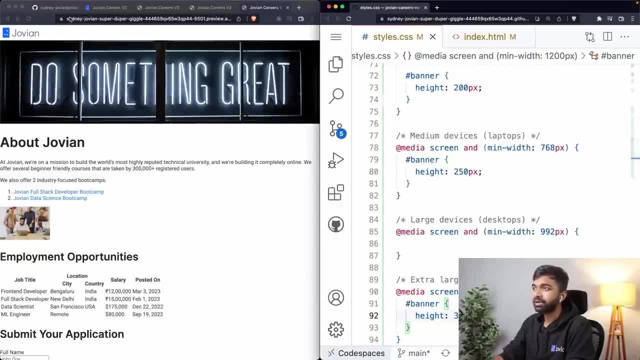 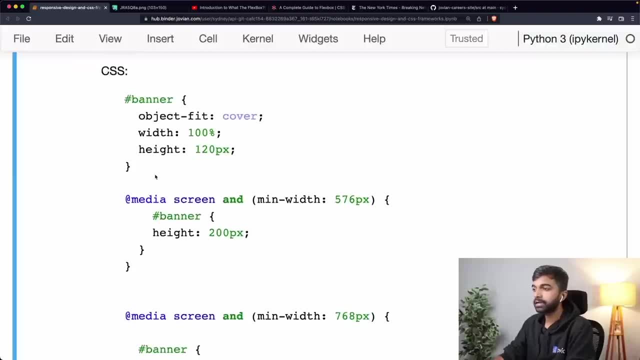 bigger. All right, So that takes care of the banner. I don't think there are any other changes required. So we've removed the height property that was there on the image and we've actually said I'd specifically add various breakpoints. So it's going to start out with 120 pixels. 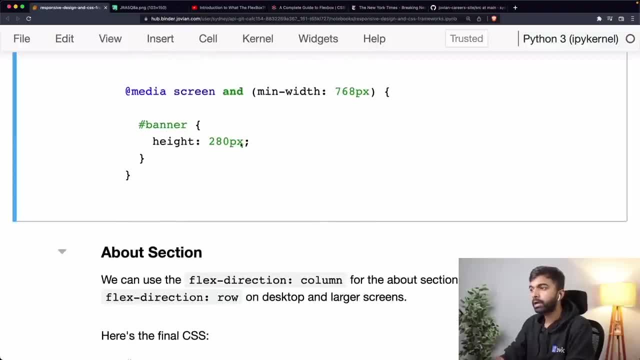 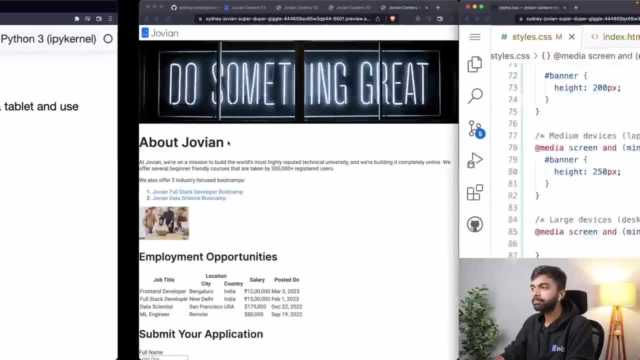 It's going to grow to 200 and then to about 280 pixels or so at the desktops. That was pretty straightforward. Let us now go ahead, and let us now do the about section as well. This is the about Jovian section. 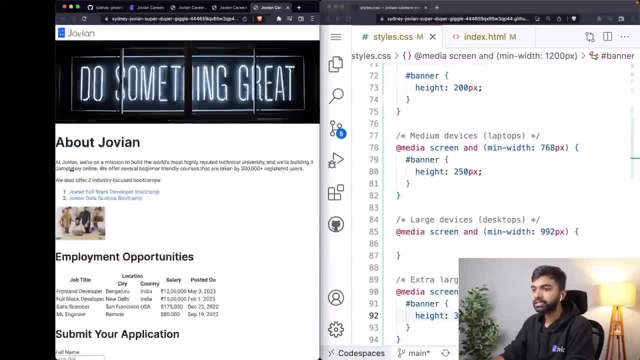 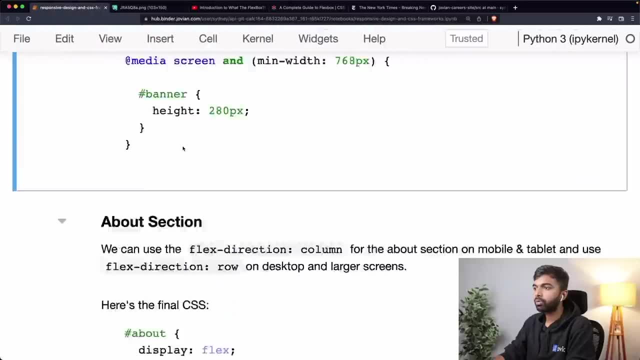 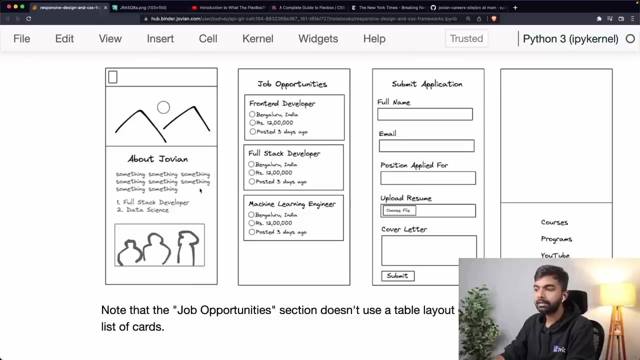 It has this edge one, and then it has some text over here, and then it has this image as well. And what we want is, if I go back to our layout, we want the text to show up above the image, still centered, but on desktop we want them to show up side by side. 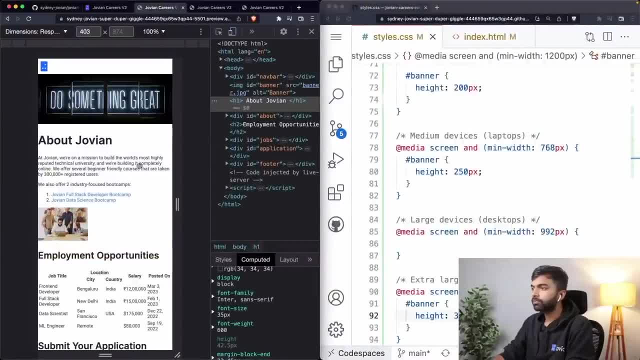 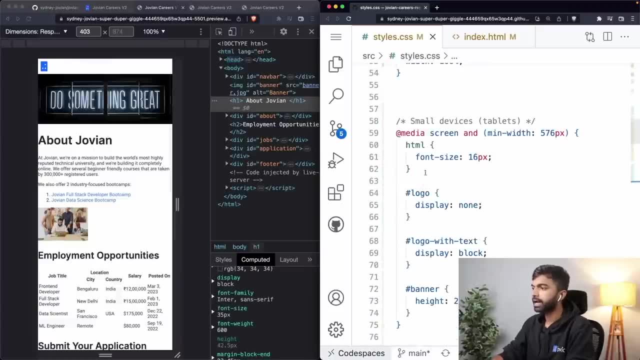 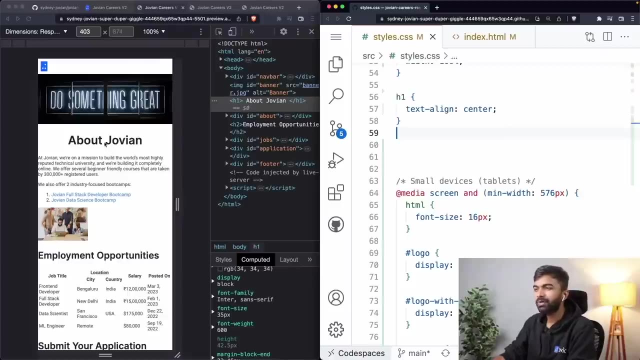 Let's try and achieve that. The first thing I'm going to do is just copy over the styles for each one, So each one has text align center. That's good, I'm just going to keep that Okay. But I feel that the space here above and below each one it seems to be very high. 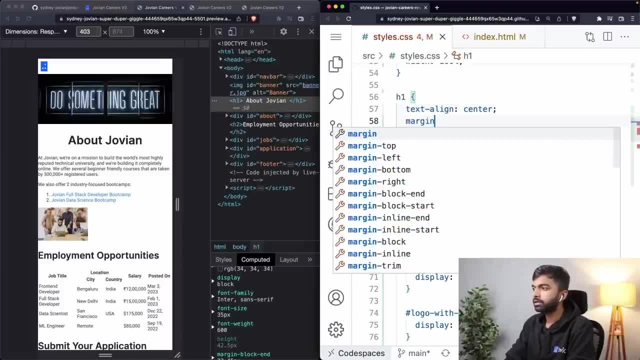 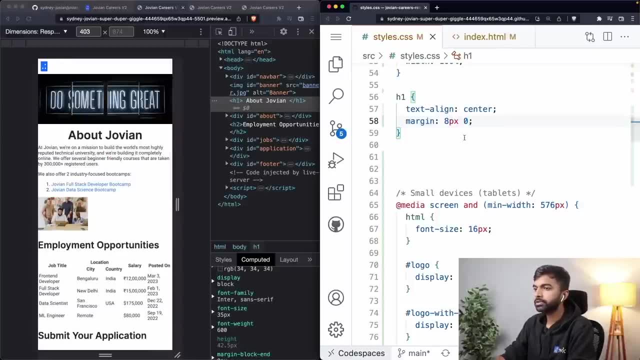 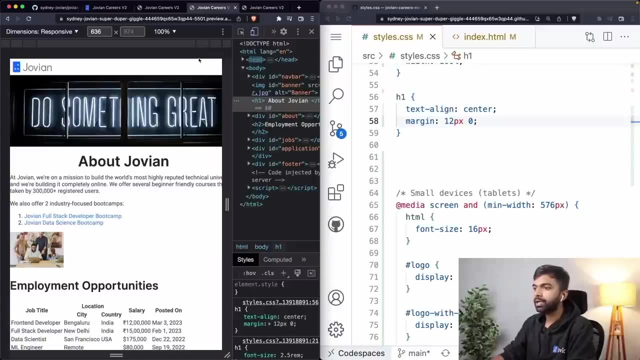 So I want to reset that. I just want to say margin. I just want to set the margin to eight PX zero. So just eight pixels of face above and below would be good enough for me. Maybe I could go 12 PX. 12 PX looks fine, but of course that may not look good on tablet. 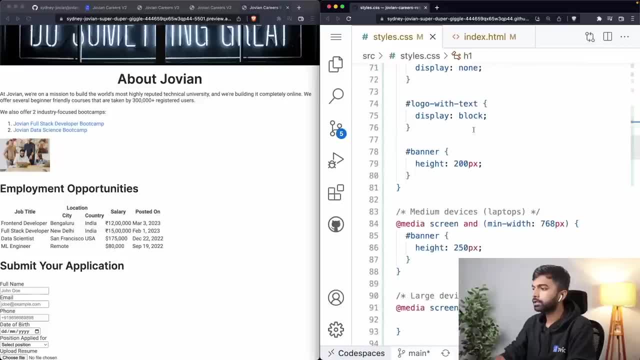 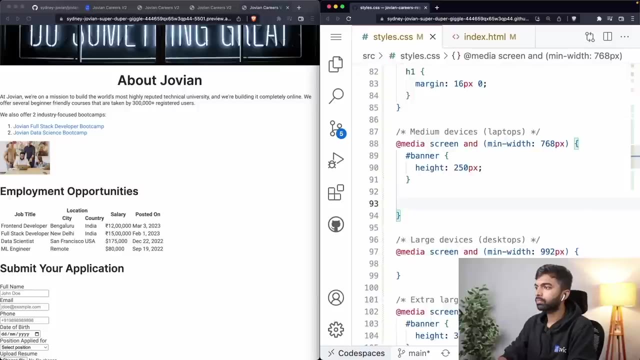 and on desktop. So I might then have to go in here and I might need to just put in an edge one. Okay, So margin, let's say 16 PX on tablet, And I might go in here and into desktop and I might set margin to 20 PX. you know it's. 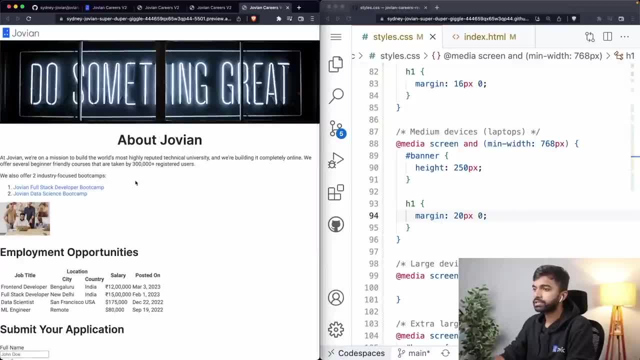 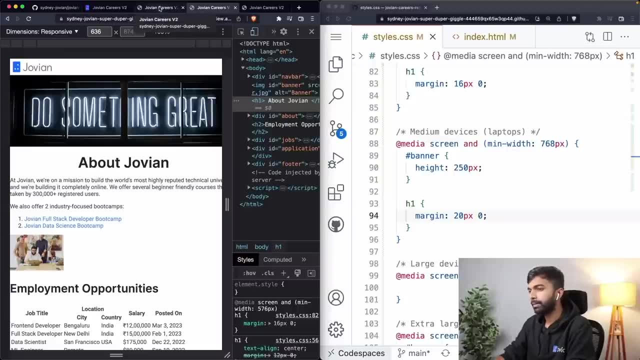 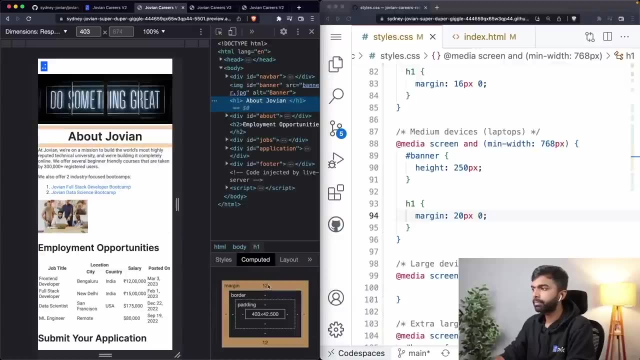 about 20 pixels on the desktop, which looks fine, About 16 pixels here On mobile, on pad, on tablet, that looks fine, And about eight pixels here, And I can verify this. I can click, inspect, I can go in here into the computed styles and make sure that it has the right belief. 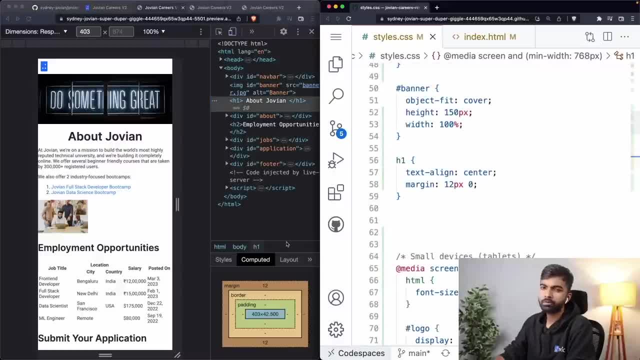 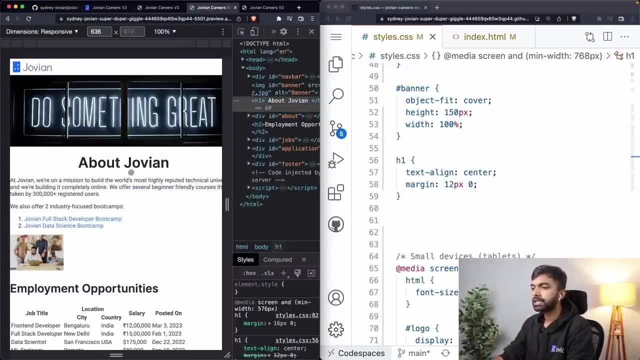 Well, pixels is what we put here, So 12 looks fine. Okay, That's how you can progressively enhance spacing or the edge one, but otherwise this looks fine to me. Of course, the edge one itself is also bigger because of base font size is bigger. 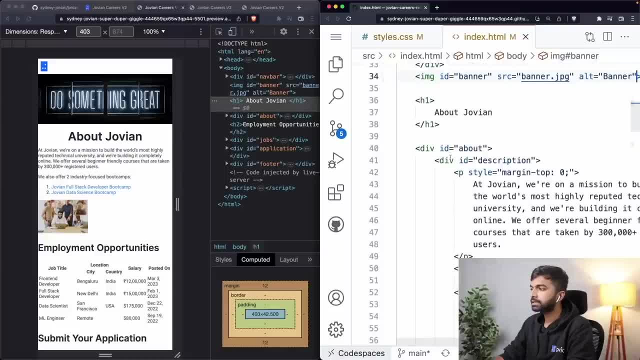 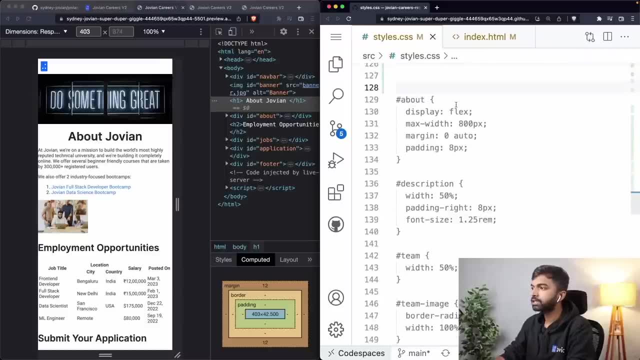 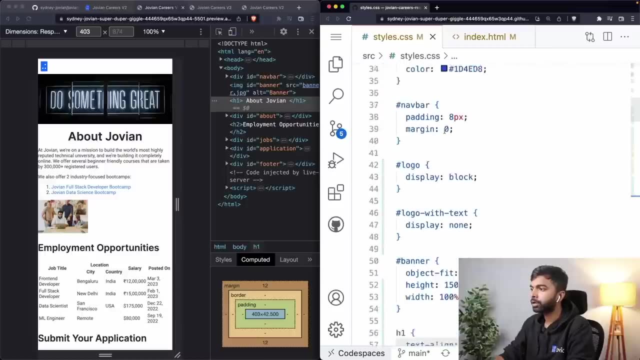 Okay. Next up, We have this about section Which has the ID about, and notice that we have set a don't need this. notice that we have set a maximum width for this about section. Okay, So we may not need this maximum width on mobile, but it was. it is still useful on tablet and. 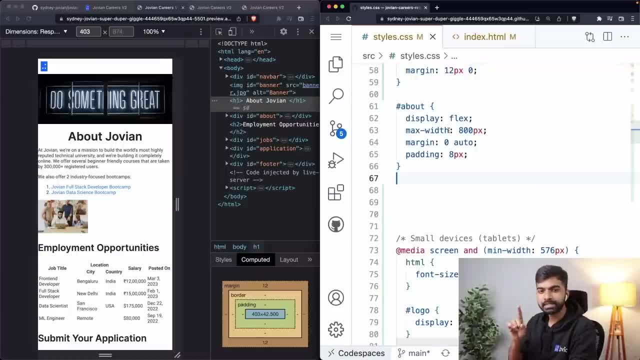 on desktop, So I'm going to keep it around. So you want to use display flex? that is, that was for the horizontal layout, And then we have given it a max width of 800 pixels and we've given it a margin zero, auto. 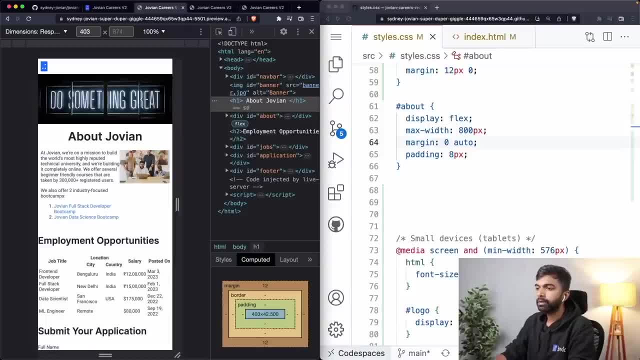 and we've given it an internal padding. Let's just check, Okay, So now, as soon as we did this, you can see that here it has taken up some space and now it is showing things left to right. Here is what I can do. 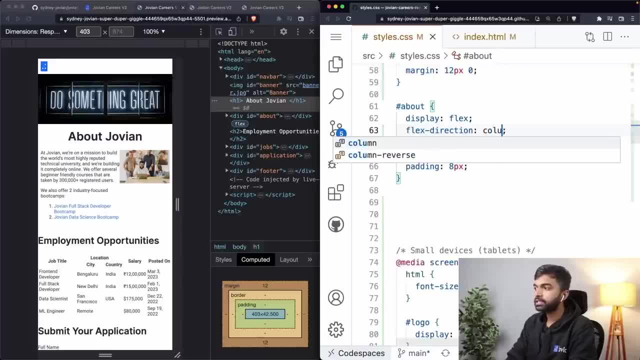 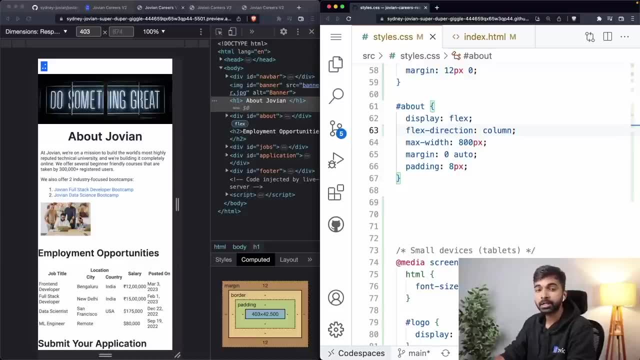 Now this is the benefit I get with flex: I can just set flex direction column, I can use flex direction column. So that thinks the first and the second section, the description and the image one below the other, and then I can go in and let me see what I want to do for tablet. 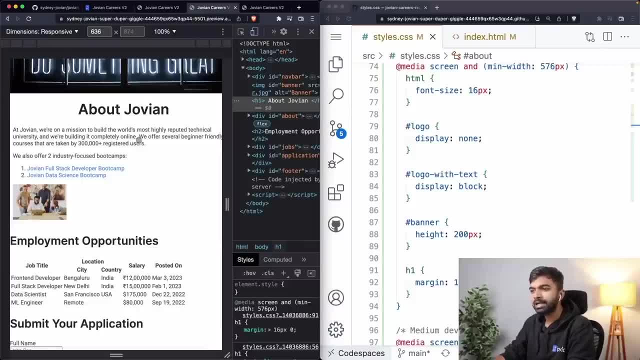 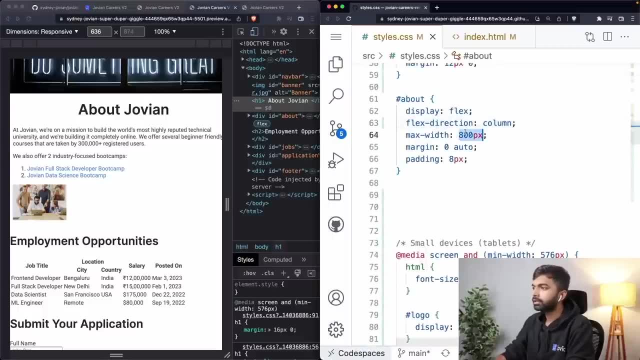 So for tablet as well. Okay, So I think I want to keep this layout, but I want to limit the width to about 500 pixels. I don't want it to go all over the place. So I'm just going to put in your max width of 500 pixels so that on mobile and tablet, 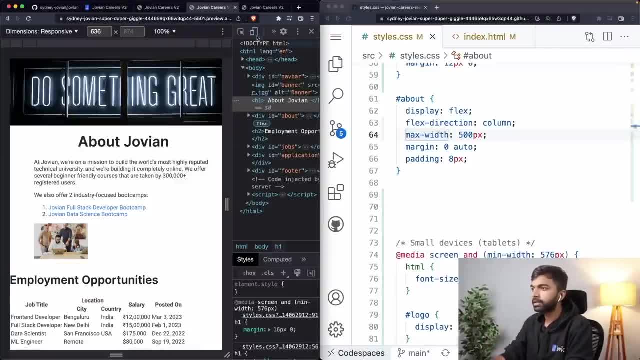 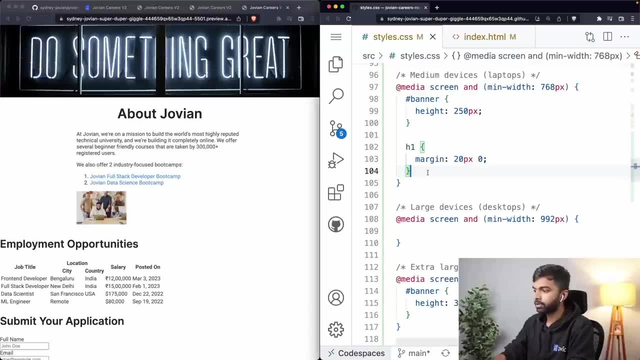 it just uses 500 pixels. on tablet Also, this looks fine, but definitely on desktop I wanted to take up 800 pixels, as it is available. Right, So I'm going to go in and I'm going to say for the about section: 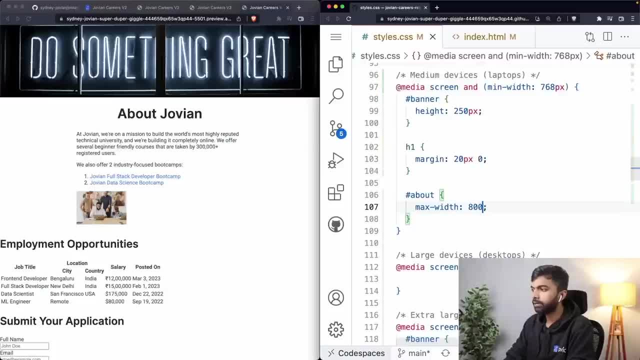 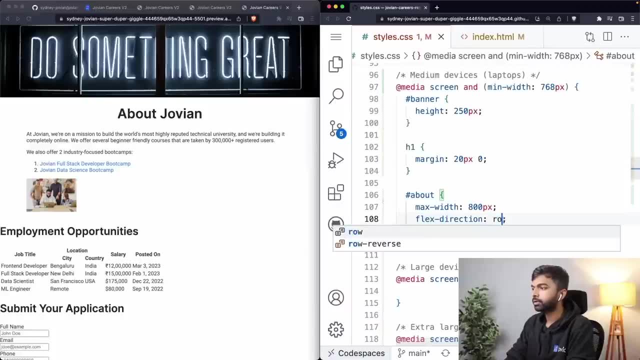 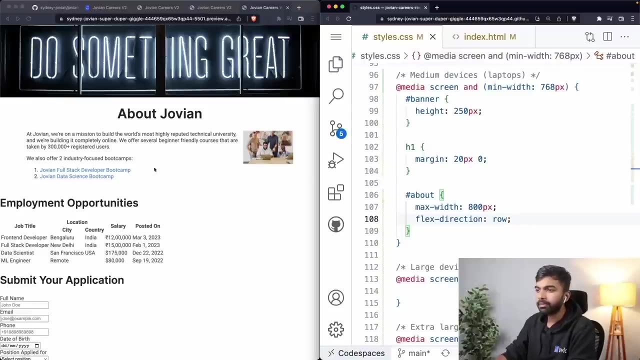 Set the max width not to 500, but to 800 pixels. So now it's taking up 800 pixels and set the flex direction to row and not column. So now it's going to show up side by side. Okay, This is great, but of course it's not taking up 50% of the space. 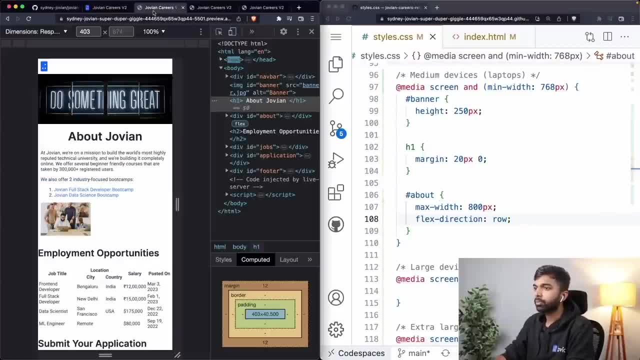 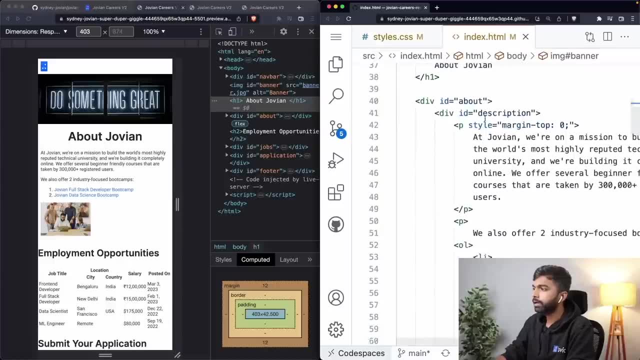 So I need to fix that as well. So let's come back to the mobile view. Now. there are two parts within about. there is the description And then there is the. there is a description and then there is the image- the team image. 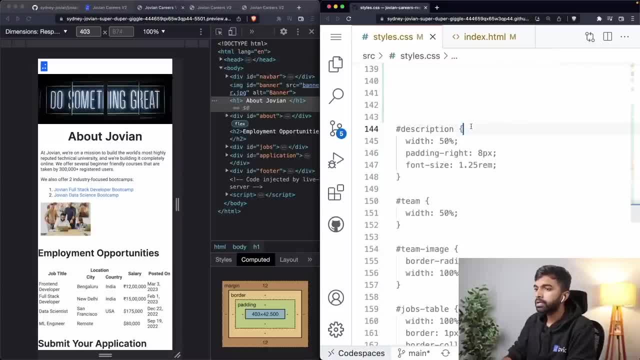 So let's first get what we're doing here before the description. we have the width of 50% that we need to set only on desktop, and we have a font size as well. So let's just copy these over and let's try to fix them one by one. 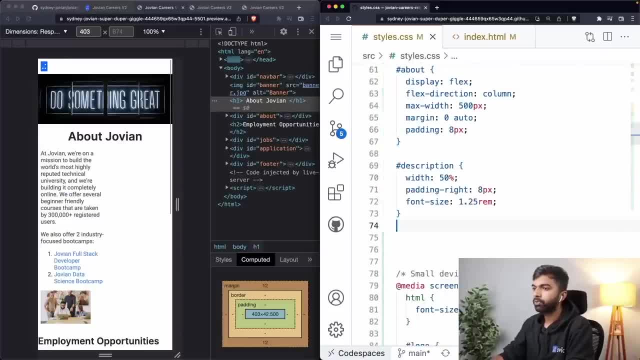 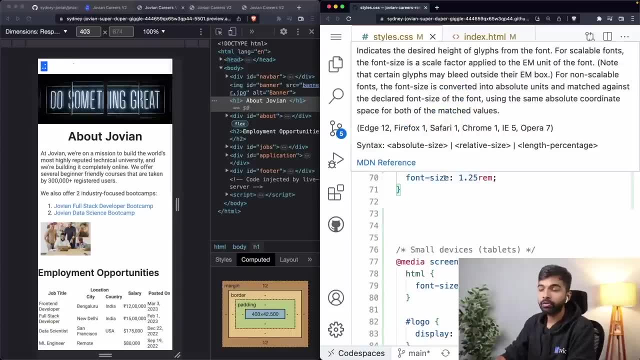 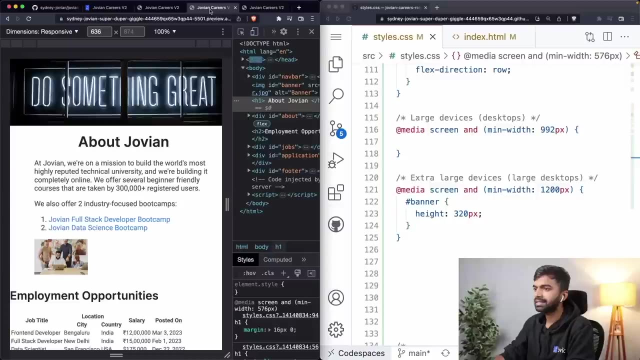 Let's see: here We are going to use the description. We don't need width, 50%, Okay, And we probably don't need the padding, right, But we do want the font to be 1.25 rem. So I'm just going to come in here and I am going to go into, maybe the large device, because 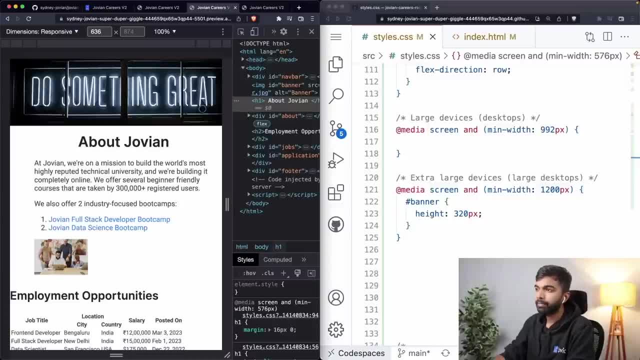 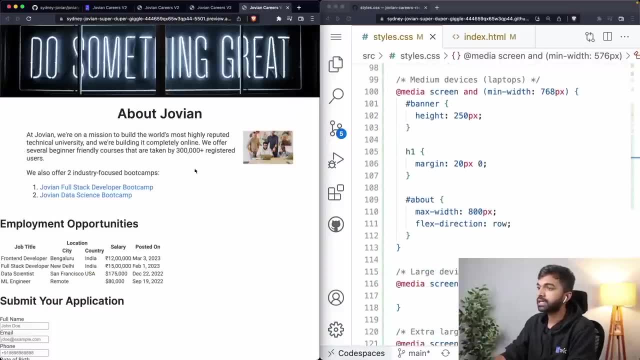 I think this still works for the tablet layout as well. I'm just going to go into the large devices. I'm sorry, I'm just going to go into the medium devices. which is more than 768 pixels, which is what this is. 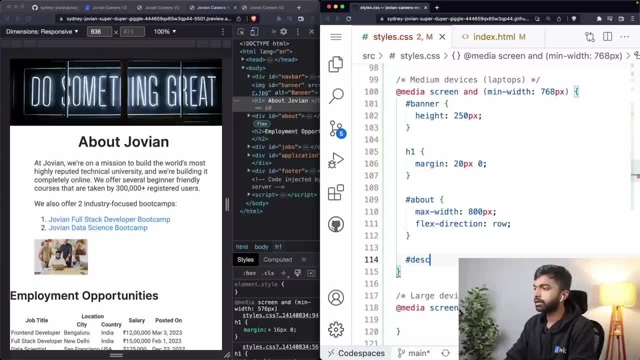 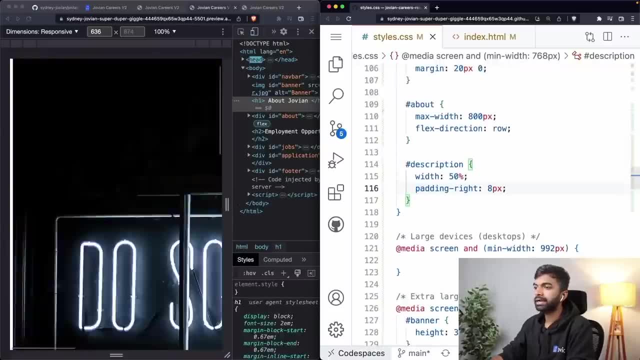 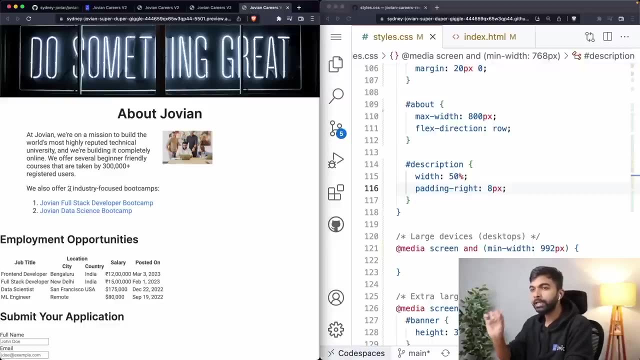 And I'm going to add the width condition here under description. Okay, Let me add a width of 50% and let me add that padding right so that there is space between the description and the image. And now you can see here that the description takes up half the space only on the laptop. 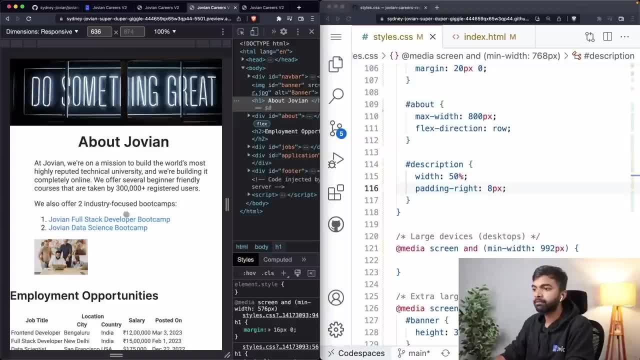 desktop and all the bigger screens It doesn't take up. it takes up the full space on tablet and it takes up the full space on mobile as well. And of course, the flex direction also changes from column to row, And that is why the rest of the space is taken up here by this image. 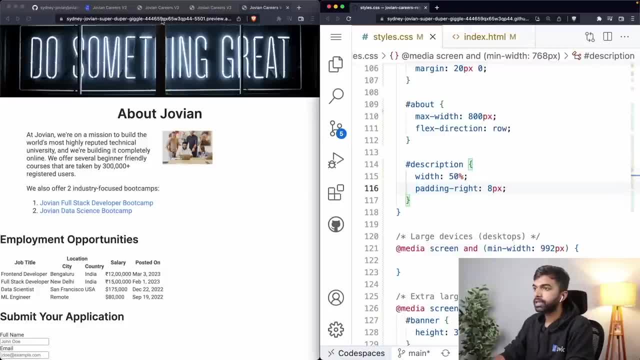 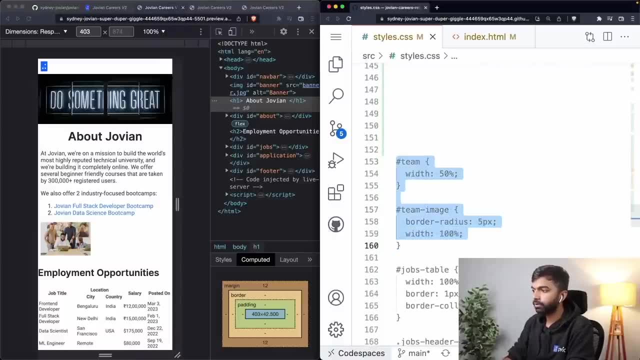 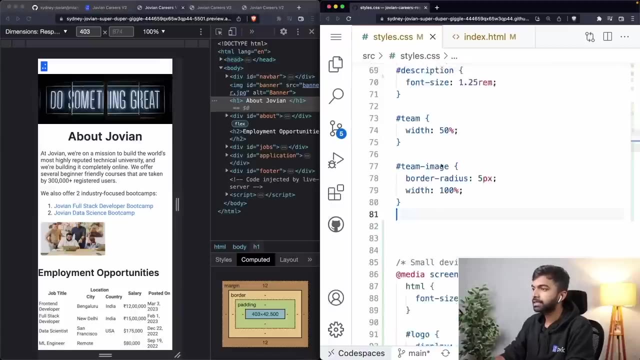 Okay, So the next thing to do is to fix this image. So let's see, we are going to get this image. So we have this team div and it's currently configured to take up only 50% of the space, And I don't think that is necessary here. 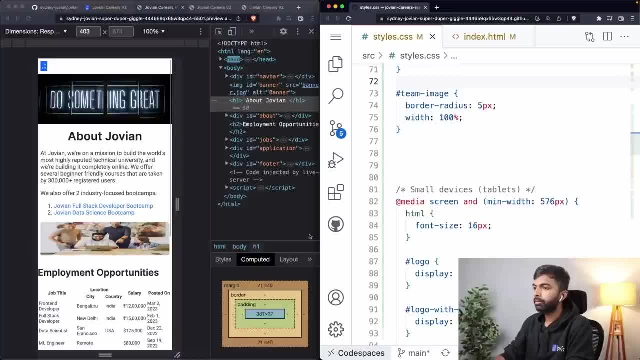 So I don't think we need to take up 50% of the space here, but I do like this border and looks like there is a height we have set. So this height is probably coming from the HTML, So Let's remove this height. 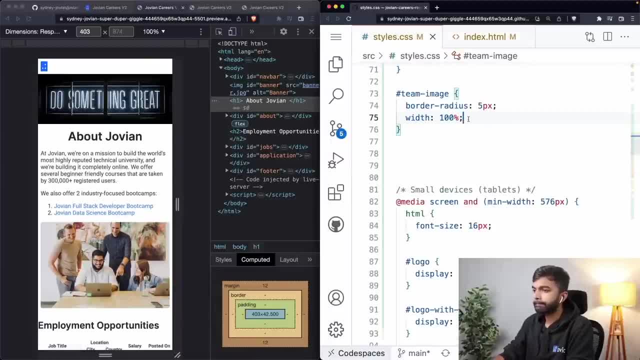 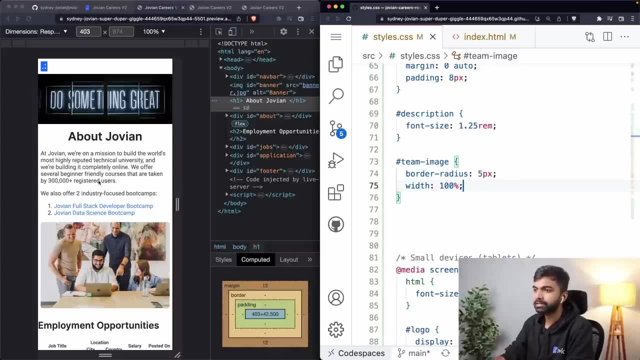 This is the team image. I think this is looking good And this has the full width. If I want, I could limit the height, but I'm not feeling like it. I'll just leave it as is. I think this image is looking good. 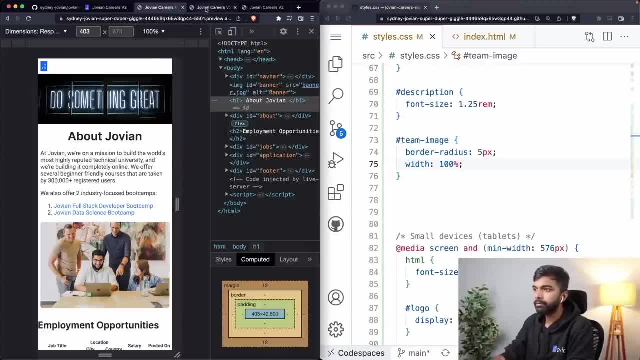 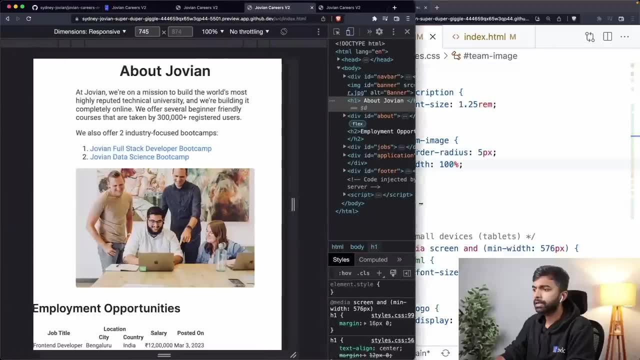 I'll just leave it as is. So it's looking good on mobile, It is looking good on laptop, on tablet as well, I think on tablet too, because we've limited the maximum width on tablet to the team image is looking fine. Looks fine on tablet. 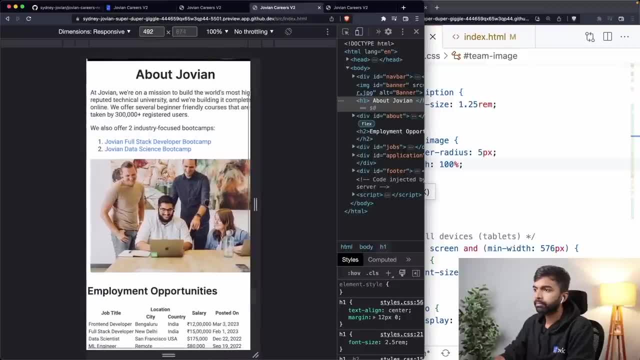 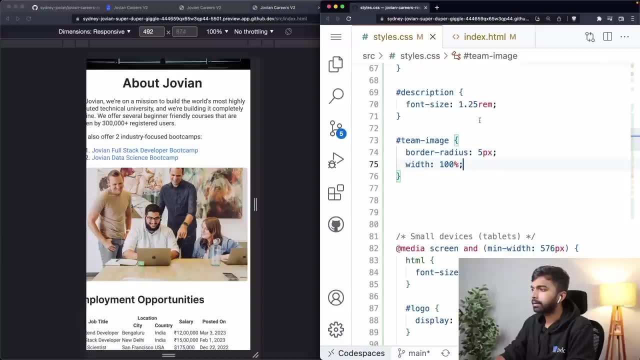 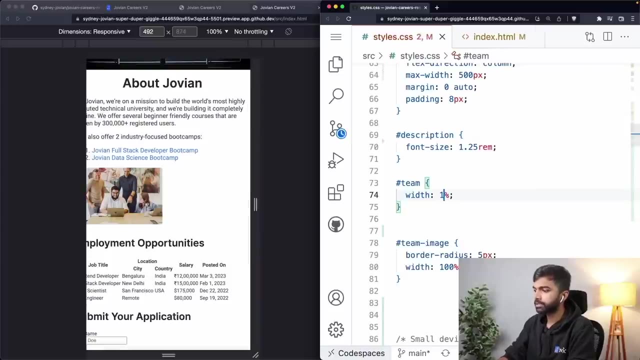 Maybe we might need to configure, like a: I need to configure something to make sure that it is actually up properly. Let's just give him a maximum width of, or a width of, a hundred percent. Yeah, a little bit, a little bit problematic. 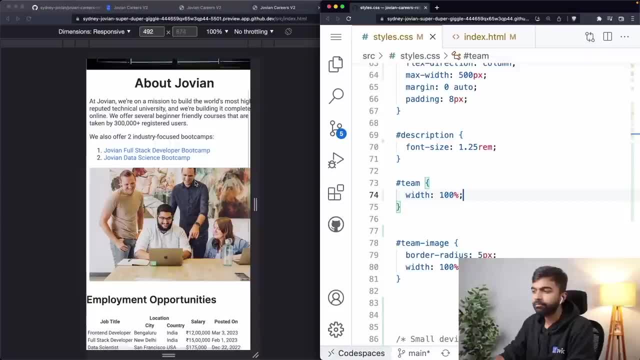 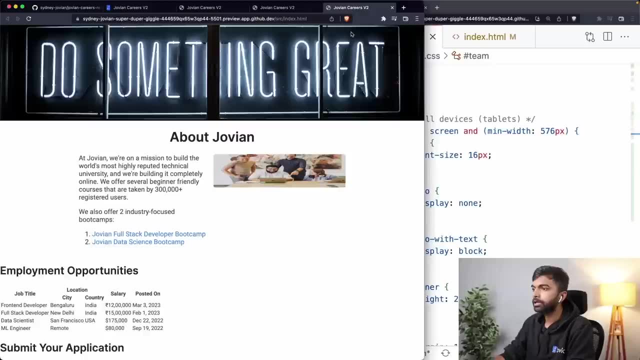 So there may be some- Yeah Yeah, There may be some minor fix that may need that we may need to do at the very end and we'll inspect it and fix it, But for now this is fine. but where we really need to make a change is over here. 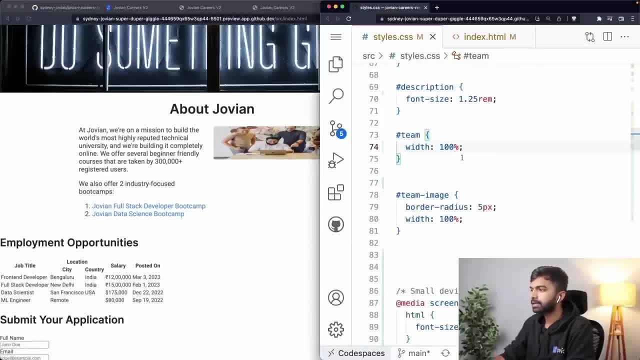 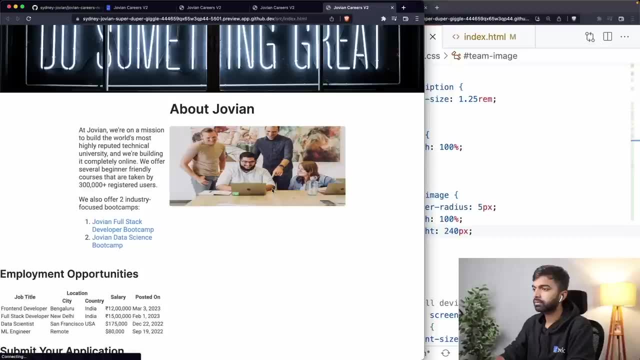 So let me do one thing. Let me just fix the height of the image as well. So let me just fix the team image height to 40 PX. Yes, we don't need it. I think this is fine. Yeah, But now it is taking up too much space. 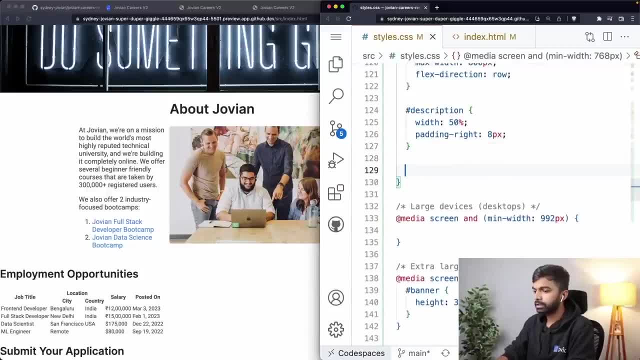 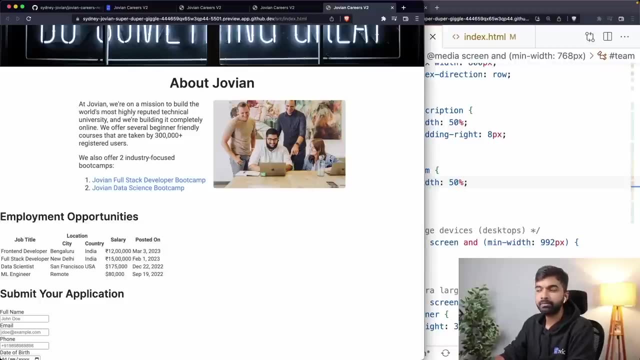 So we need to go in here And on the large desktop layout, the team did just take up a width of 50%. all right, So this is what we're going for. We have the left half, which is, and, of course, the maximum width is 80, 80 pixels, and it. 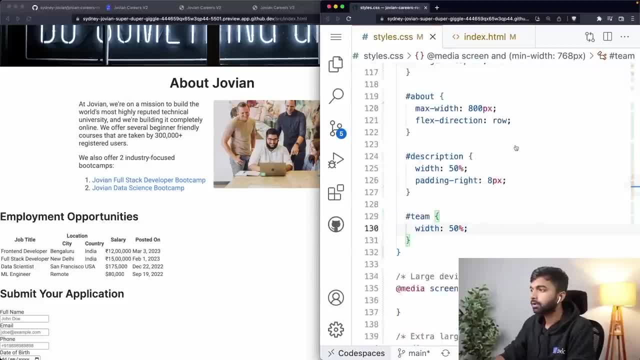 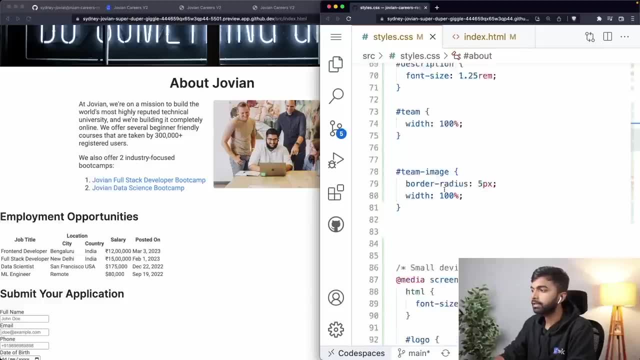 is centered vertically using margin zero auto. but that is all that is being done on the about section here: margin zero auto and max width of 500.. And then the max width is increased to about 800. here The flex direction is a row. 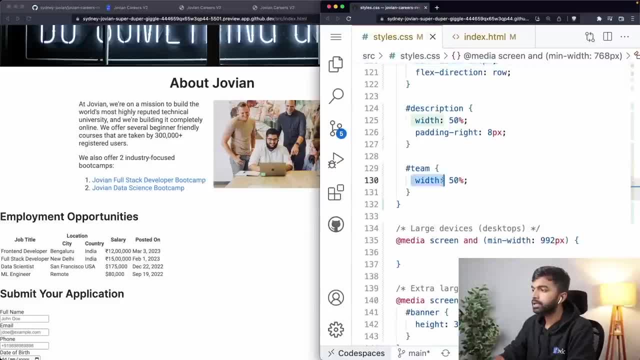 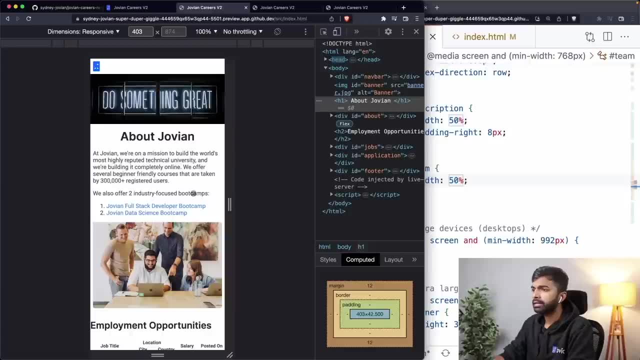 So that's why this is showing up like this, side by side, And the team image is as a width of 50%. So that is looking fine too, Okay, And it looks fine on mobile as well. on mobile, too, This team image is looking good. 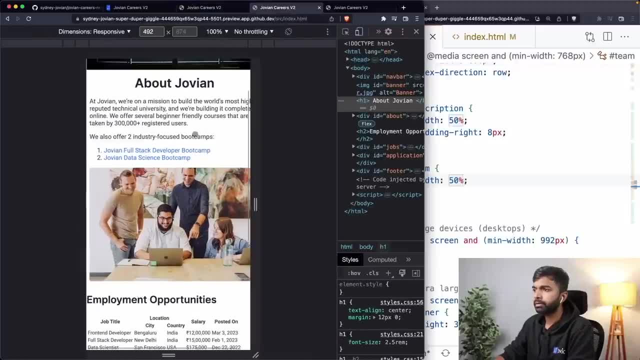 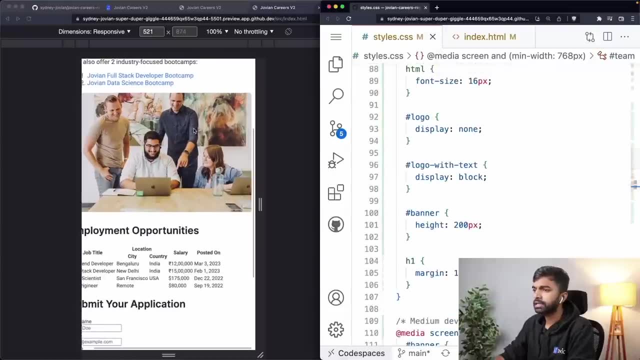 I don't see any problems here. It looks fine on tablet as well or less fine. I don't see any major issues here. We may have to make some changes. Okay, We can change later on, but otherwise this is looking fine. 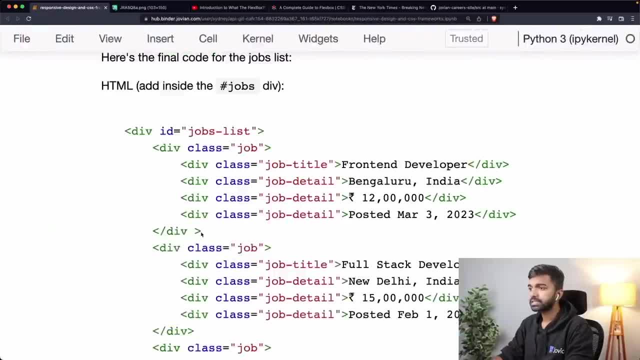 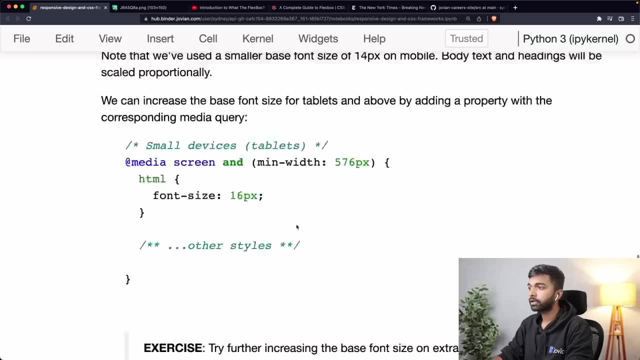 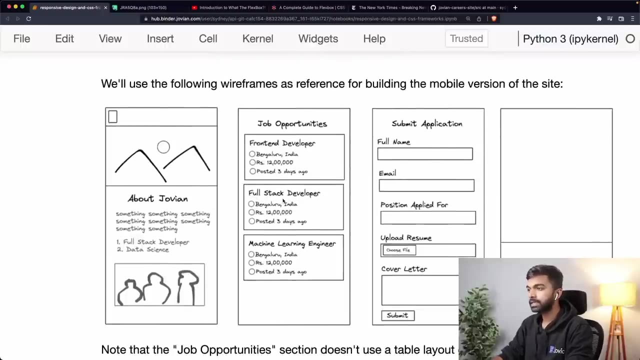 Now moving right along. the next step for us is the jobs list. Now we need to add a jobs list. Now, if I go back here, if I go back here to our mock-up on the mobile, we have a job list. So we have these cards and each card has a title and then each card has maybe one of 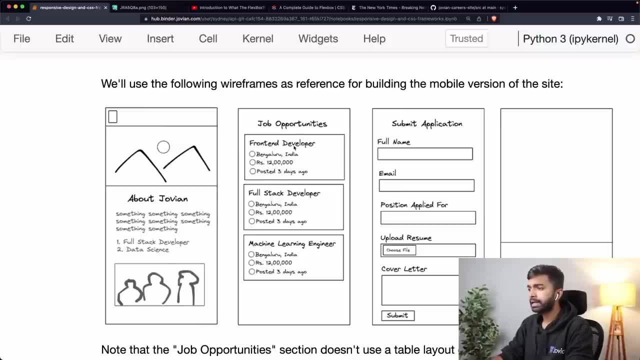 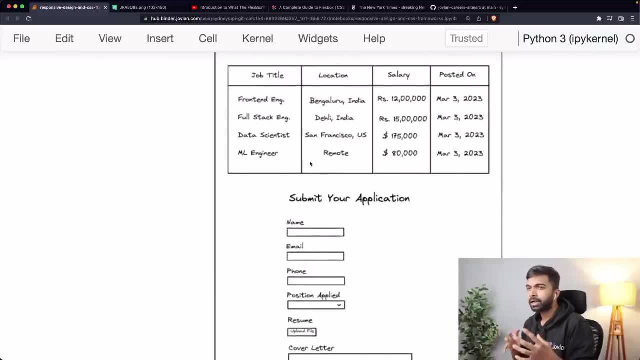 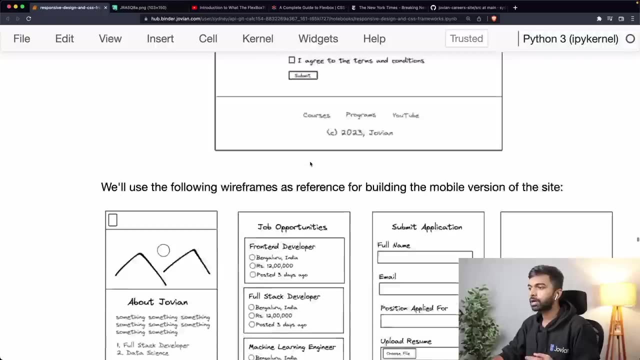 these jobs listed right And On desktop. However, we have a table. How exactly do we achieve that? We can do some kind of magic where we change the display type from div to table, and all that, But the simplest way to do it is to just show a list on mobile and hide it on desktop and 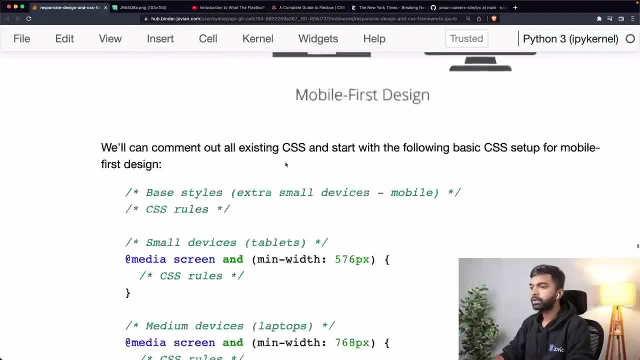 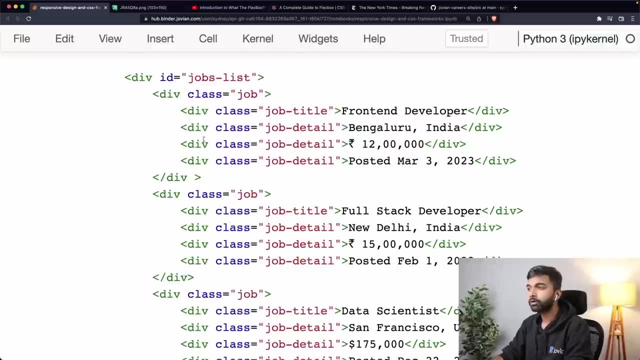 then your table on desktop and hide it on mobile. Okay, So here is what we are going to do. We are going to first take a bunch of HTML, So we're going to create a bunch of divs. So we are going to create a div called job list, and we are going to then have a bunch. 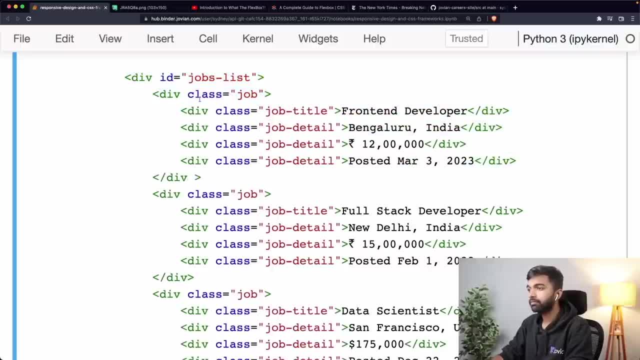 of divs, each with the class job, And then inside that div we are going to have a bunch of divs, each with the class job title for the title of the job and job detail for each detail within the job. Okay, And of course I have the data for all four jobs here. 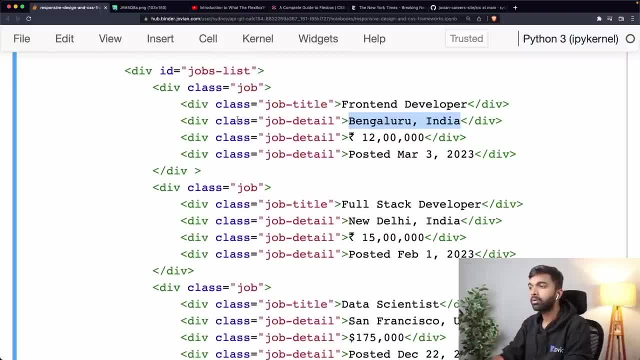 So these are the. this is the same data that is present in the table, but now I'm no longer using a table, I am simply using a. I'm simply using divs, not even a list, Okay, And I can simply copy this: 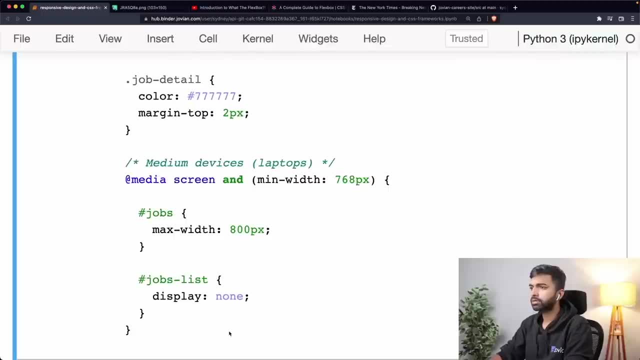 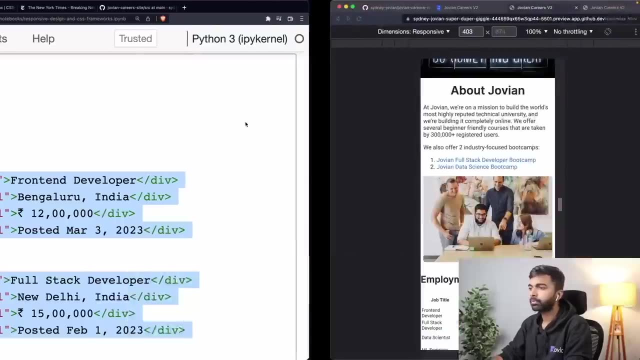 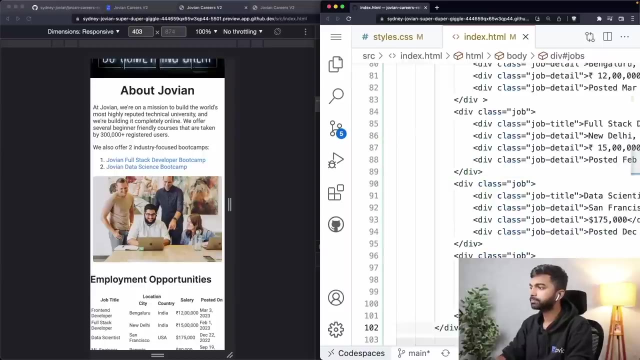 So let me just take this so that I don't have to just type all of these jobs out. Yeah, Let me just take this HTML and I'm going to go put this into my indexhtml file right under or right above the jobs table. 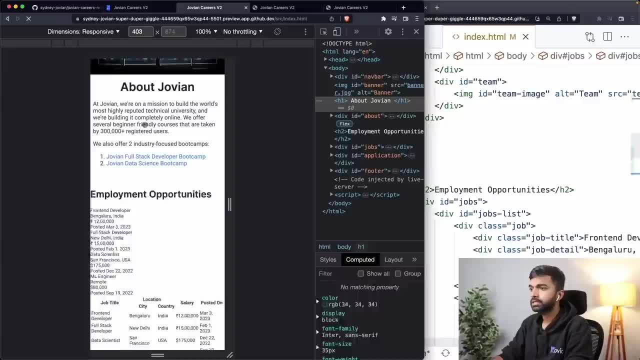 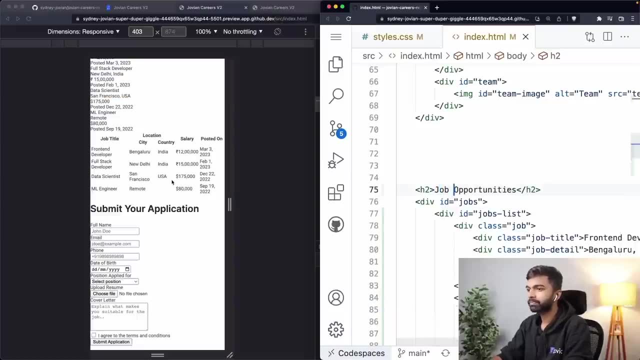 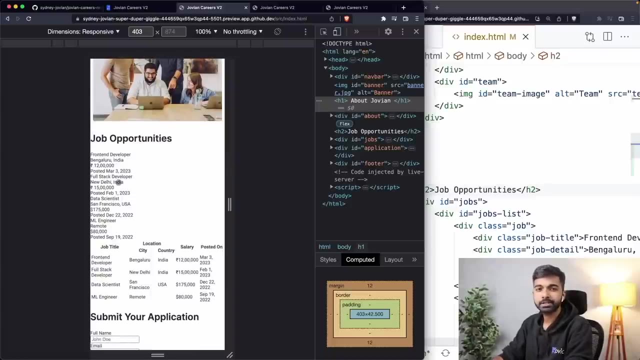 Okay, So now I have this data of employment opportunities. First let me change the employment opportunities to job opportunities. Okay, This looks better as job opportunities. So now we have this- job opportunities- and I have a list of job opportunities, which are just a bunch of divs. 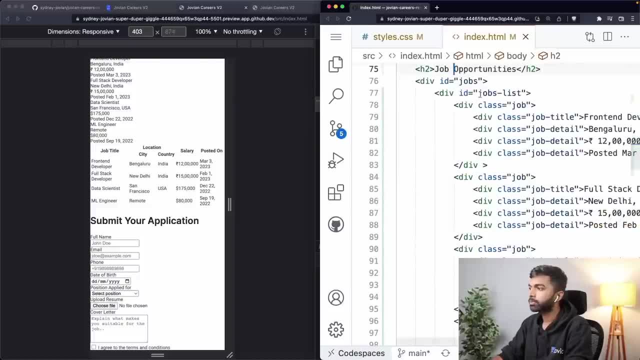 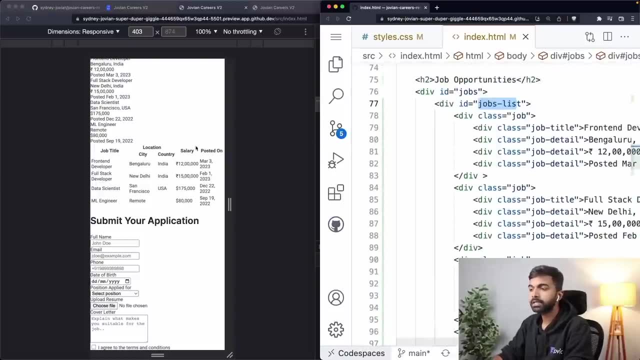 And then I have the table of job opportunities as well, And the list of job opportunities has the ID job list, jobs list- and the table has jobs table. So, as you can imagine, what we can do is we can just set display properties for both of. 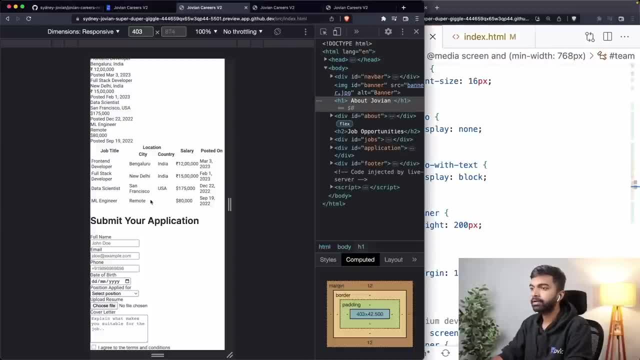 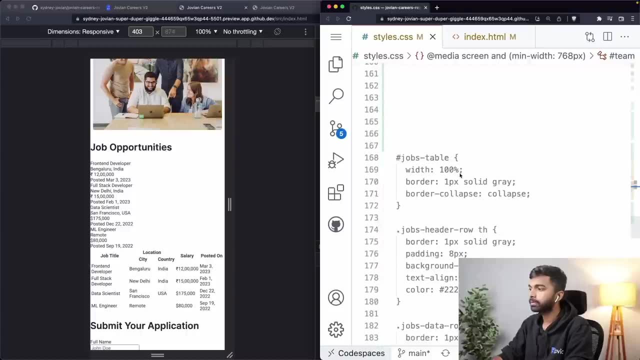 these to show and hide them respectively. And while we're at it, let us also fix the display property for this H2.. Okay, So let's go in here. Let's go down. First thing we'll do is, for the H2, we are going to set text align center. 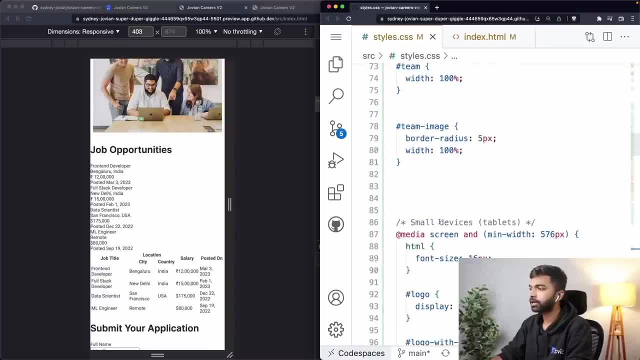 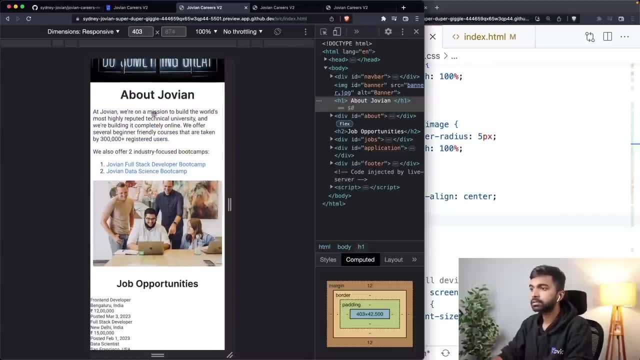 So let's bring that up. I think we are always going to have text align center for H2.. So let me just put that so that H2 has text align center. We may want to once again reduce the spacing above and below the H2.. 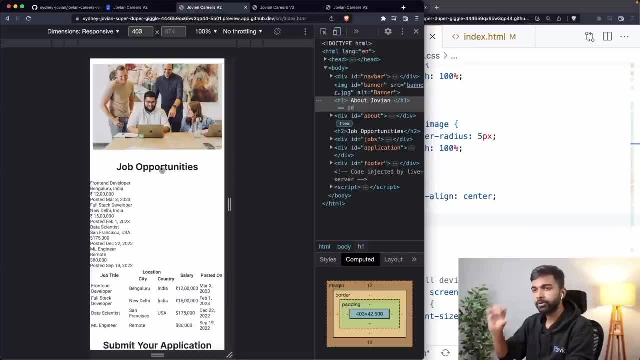 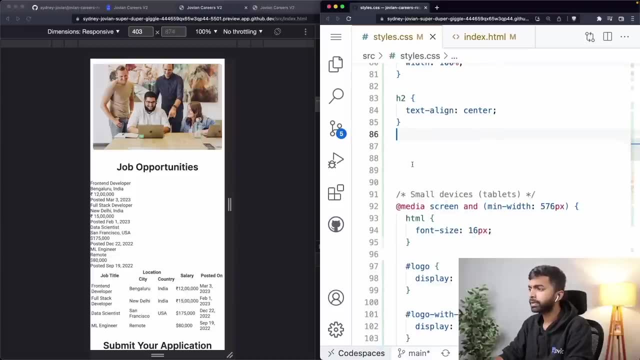 I'll skip that for now, but I leave that as an exercise. So use a smaller spacing on mobile and larger spacing on tablet and desktop Respectively. Okay, Next up, let us just figure out how to show and hide the job list. 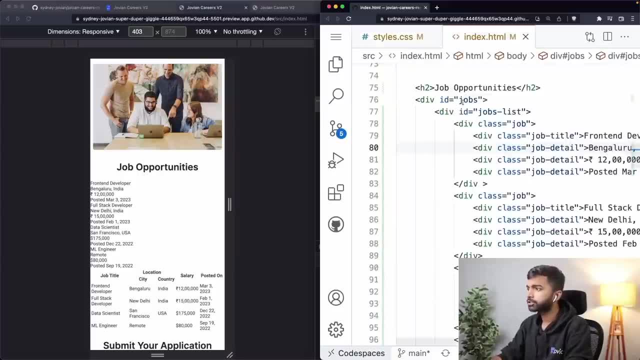 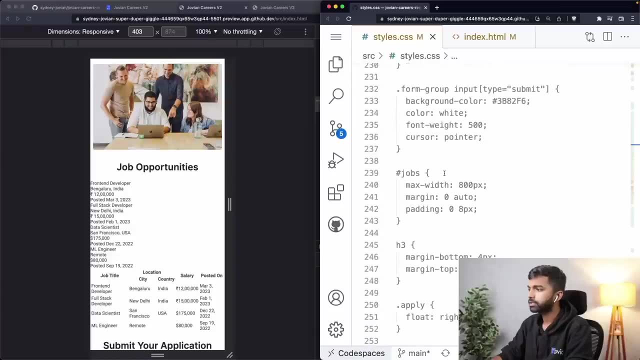 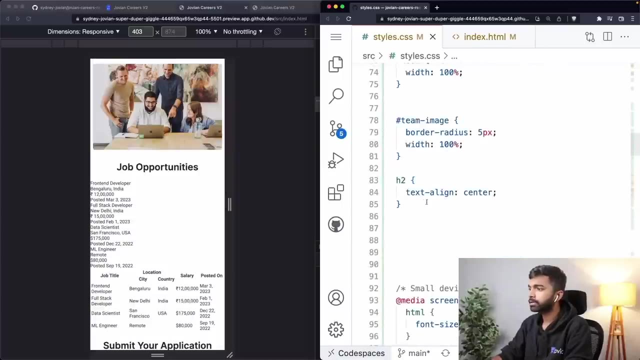 So, first of all, the entire jobs div itself. let's see if there is some setting for the entire jobs div. Yeah, So the entire jobs div has a max width of 800 pixels. Let's just take that and let us just put it here at the top. 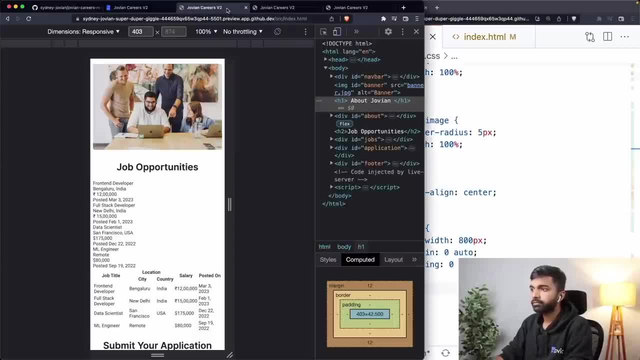 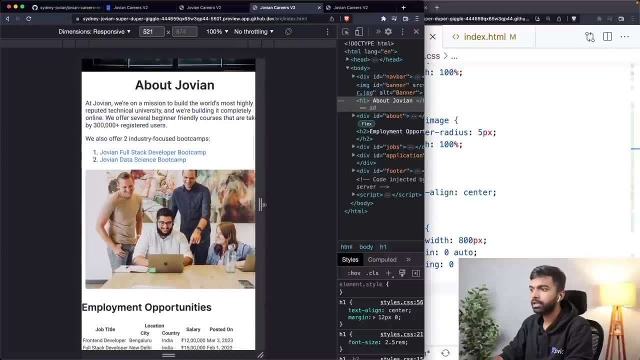 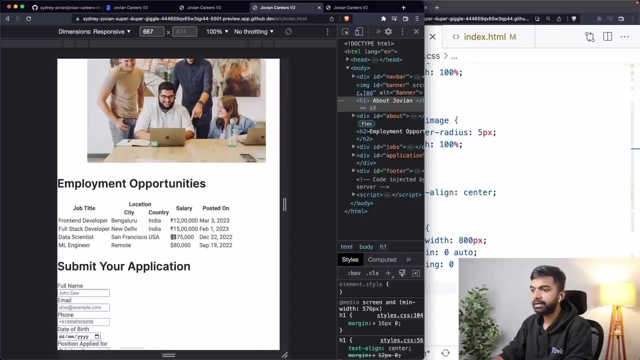 Okay, So the entire jobs div on mobile just takes up the entire width. No issue. On tablet it takes up the entire width as well, but we might want to limit its width slightly. You can see here at around 600 on tablet, we might want to just center it. 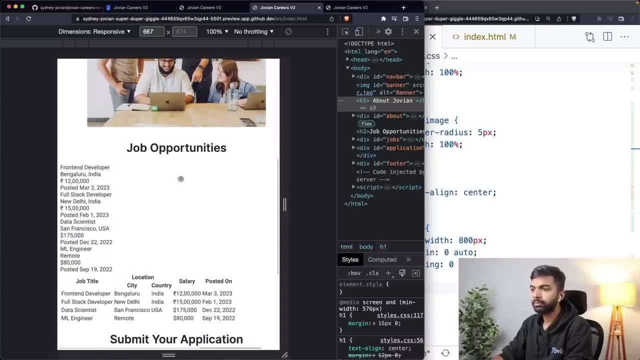 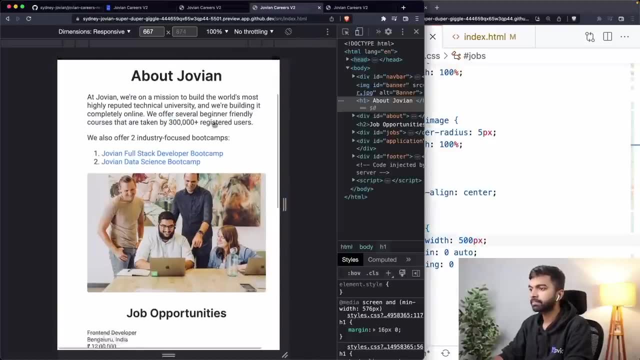 We may not want to just show it, We may not want it to take up the entire space, just like this content is centered. We may want to center it. So how about we use a max width of 500 pixels, just like that, so that the content is centered? 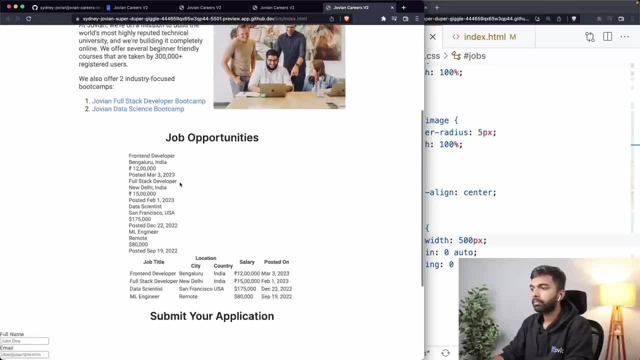 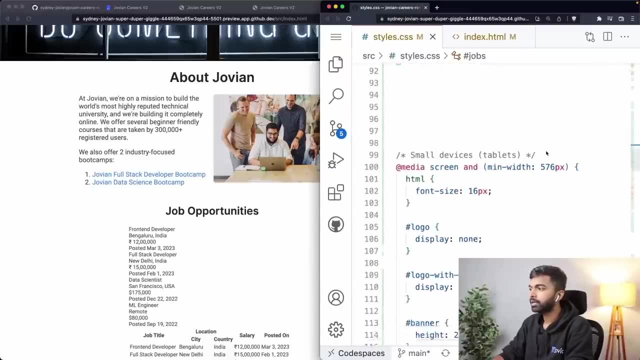 on the tablet, but then on tablet Desktop, we want it to take up slightly more width, right? So this is going up to 800 pixel width. So I'm going to come in into the desktop media query, which is laptops desktops and which. 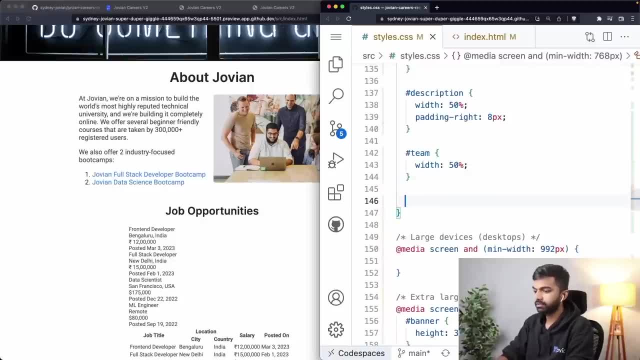 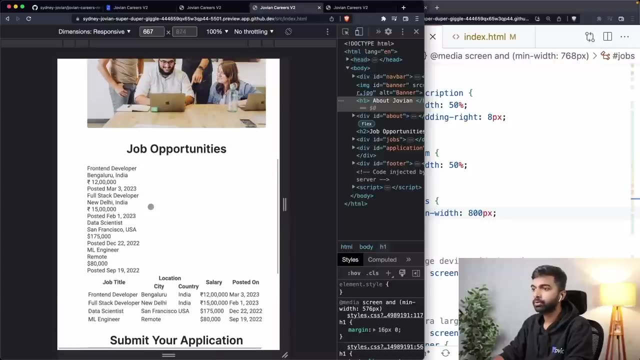 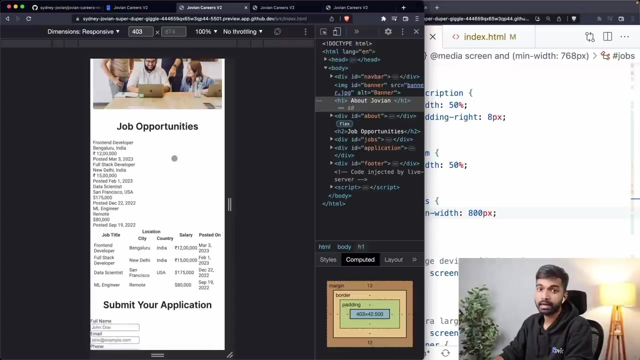 is about 768 pixels And for the jobs div, I am going to set min width of 800 pixels. Okay, Now you can see that it takes up 800 full pixels on the on desktop. on tablet it takes up only about 500 pixels, and on mobile it takes up the entire space available. 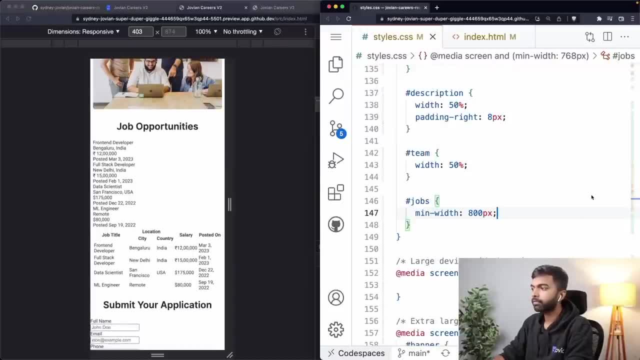 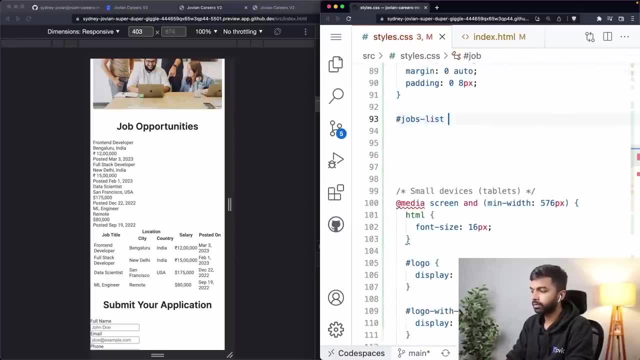 Okay, That's good. That is not set the display criteria for for both of these. I'm going to go in and there is this jobs list that I have, which I want to have display block by default, and the jobs list, the jobs table. 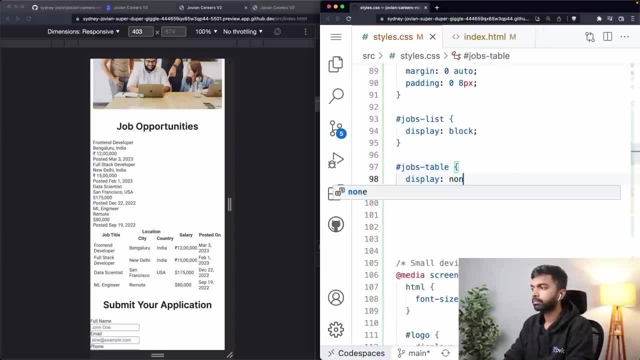 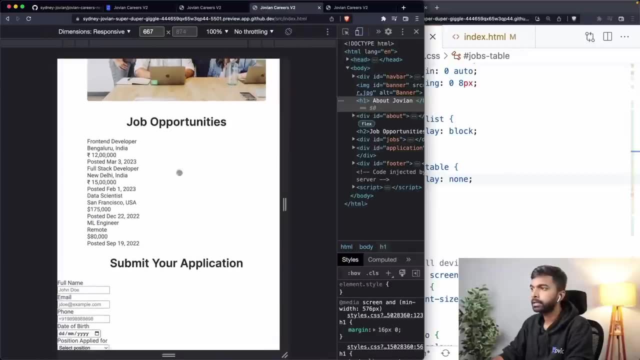 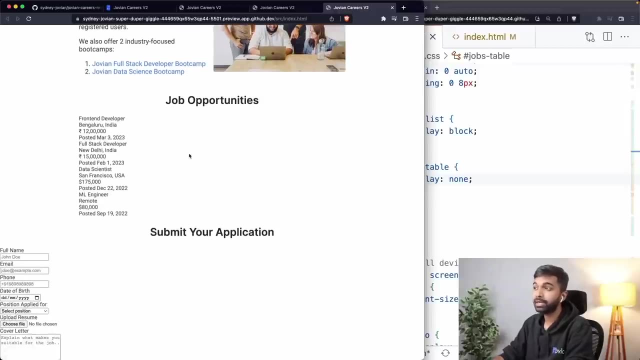 I want to set its display, So none, Okay. So now my job opportunities is visible here on mobile, It is visible on tablet and it is not visible, and it is visible on desktop as well, And this is where I may need to change something. 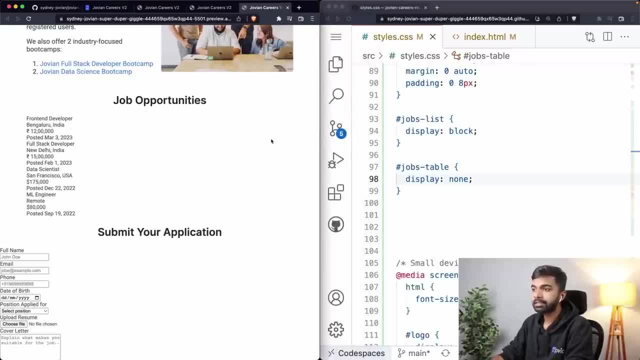 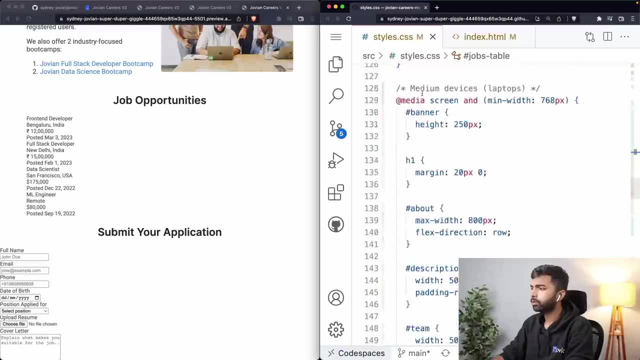 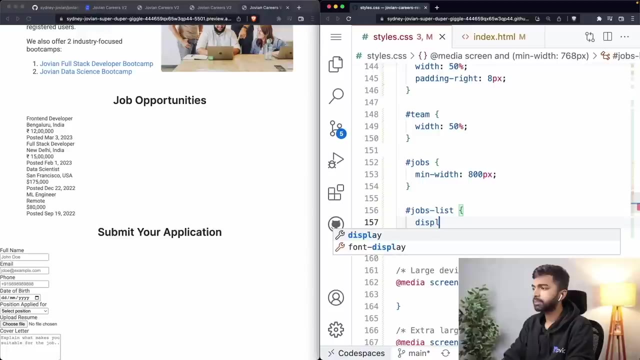 So I need to change the layout here and I want to hide this and show the table. So let us try and hide this and show the table. Well, so if I go in into this layout above site Okay, 7, 68, I'm going to say jobs list display none. 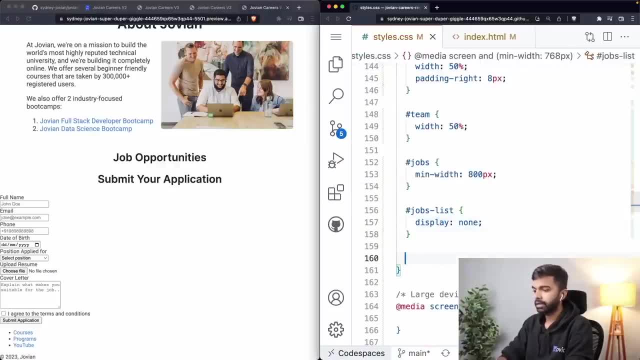 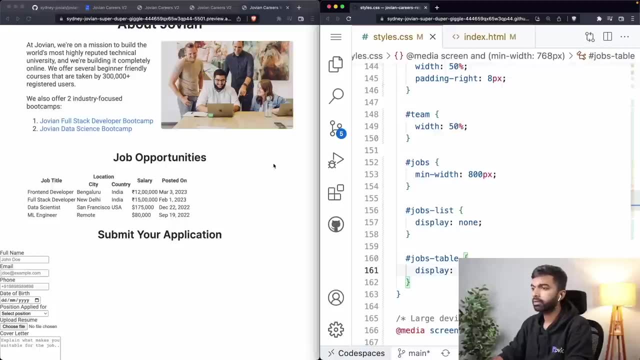 Remember, the jobs list is simply the list of jobs that we have. So that's gone And I can say jobs. table display block. Okay, Now we don't actually want to use display block here, The default value of display for a table tag. 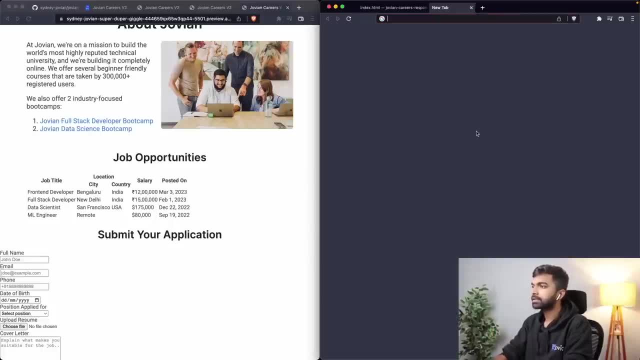 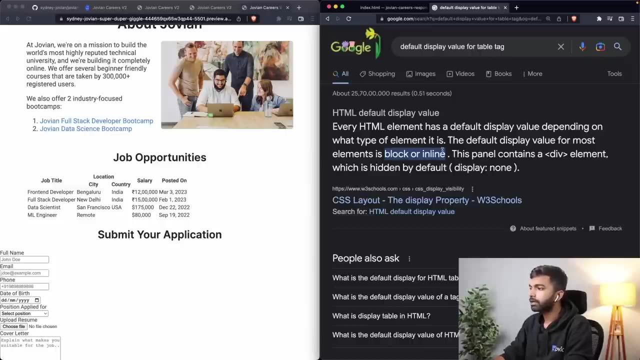 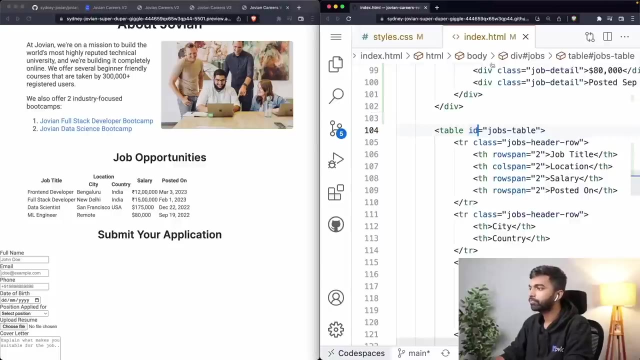 Remember, jobs table is a table. you see, here it's a table tag. Okay, Default display value for table tag. The default display value for the table tag is all right. I'll just tell you: the default display value for a table tag is actually table itself. 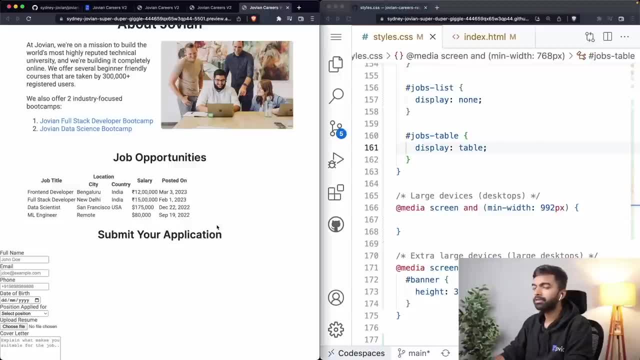 So we can. we should need to set display table here, And when we set display table here, what it does is that allows the table to take up the entire width of the screen on most, on most screens, And that will happen once we add some of the other table styles as well. 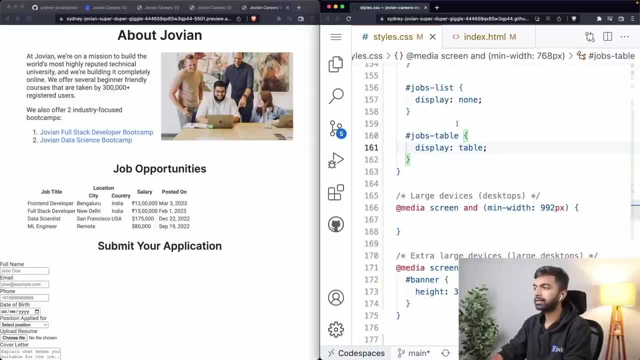 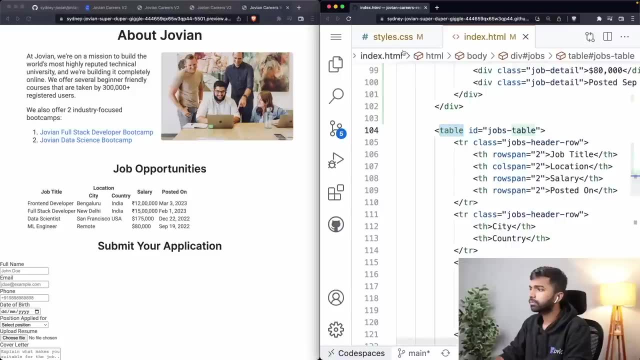 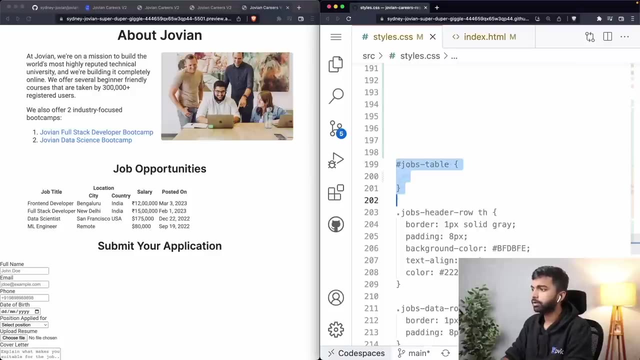 Okay, So just keep that in mind- that the default display for a table, a table tag, is table. All right, Well, we are doing fine so far. We might need to copy in where, as soon as the table is visible, we want to use it. 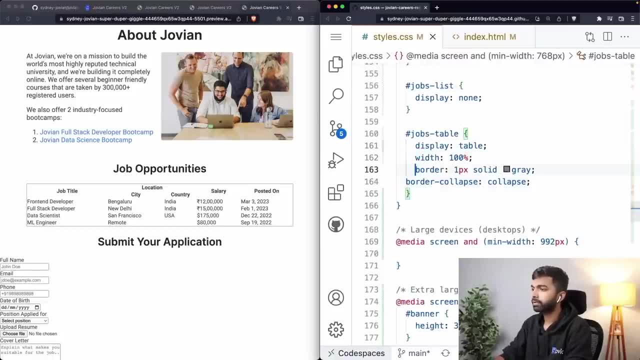 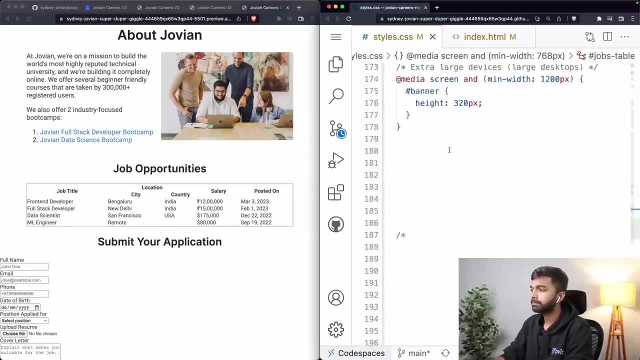 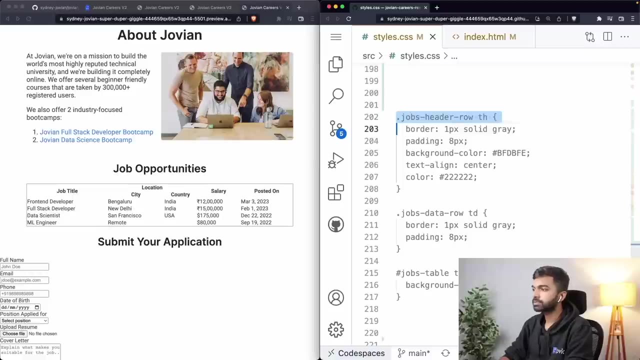 We want to set its display to use the entire width. and yes, we have a bunch of these settings as well. We have the border setting, We have the border collapse setting, and then, of course, all the table styles can be incorporated directly into the media query, where the table becomes visible. 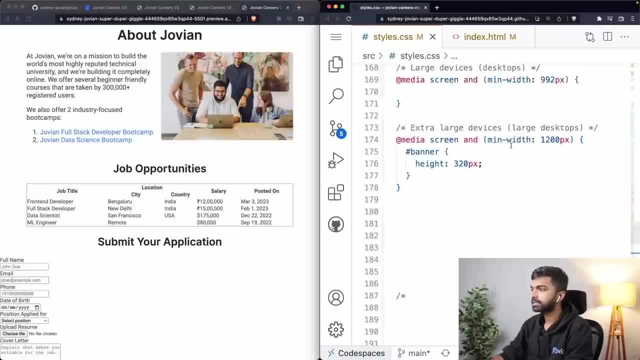 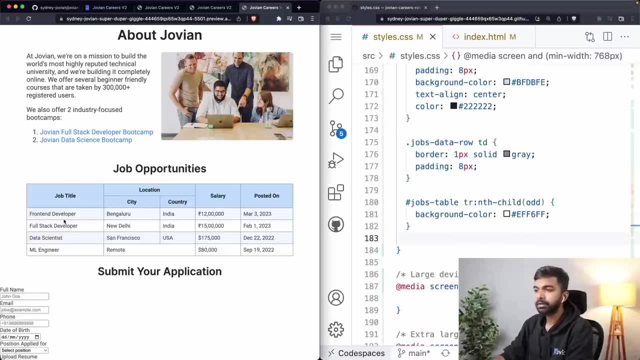 Let's capture all these table related files. So this is used to set, maybe, the borders for each table cell. This is used to set a bunch of other things. Now you can see here that our job opportunities table is showing up on desktop, but it's not. 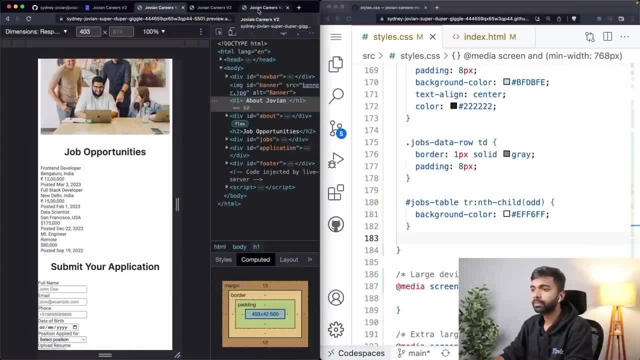 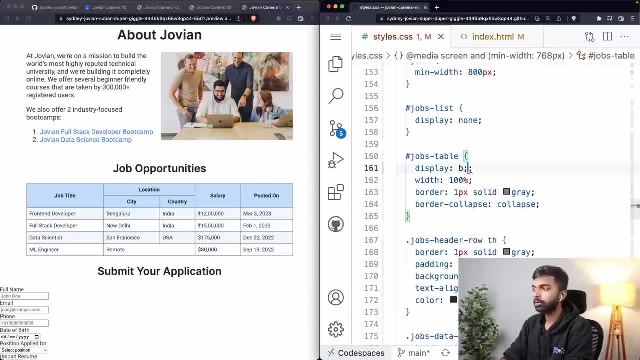 showing up on mobile. It's not showing up on desktop, It's showing up on tablet and mobile And this is because jobs table- we are setting its display to table. We can also do block, but you'll notice that in block it doesn't do what we want. 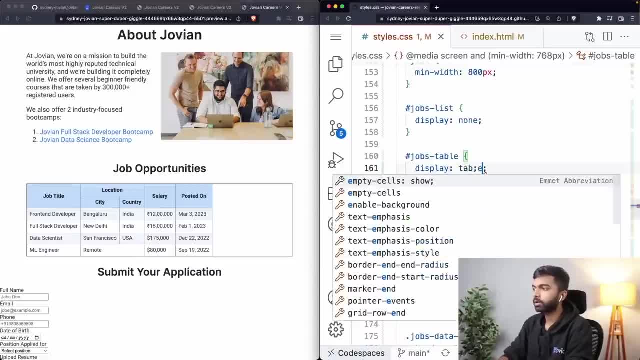 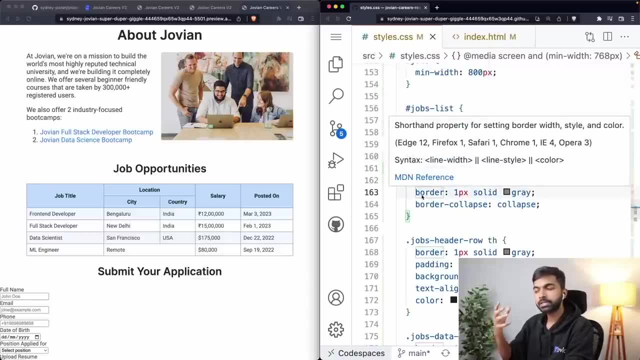 You can see that block is not what we want. We want table because we want it to use the entire available space. Okay, So display table and below below the desktop, we have this display set to none Right And of course, we have this header row. 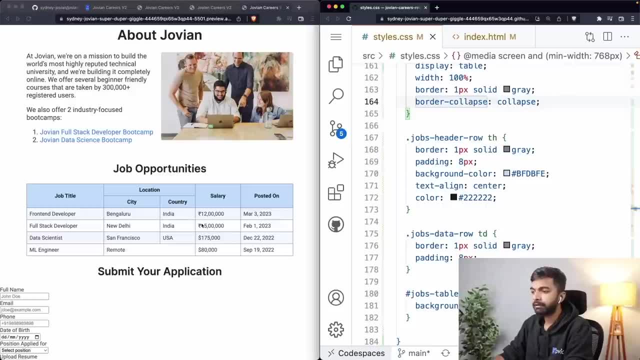 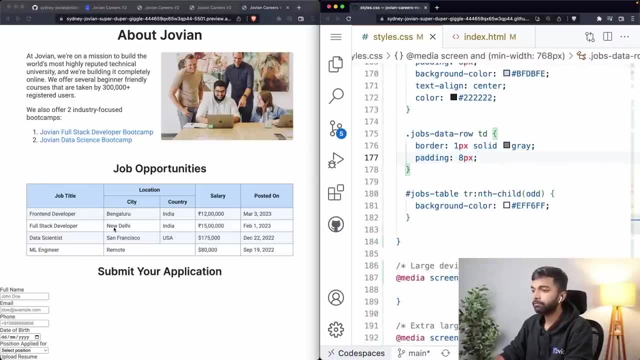 So we have colors for the header row, We have a bunch of alignments. Then we have these alternate rows. We have borders for these alternate rows. That is something that we specify here. We have a padding to space things out, And for every alternate row we also have this background color. that is done using the. 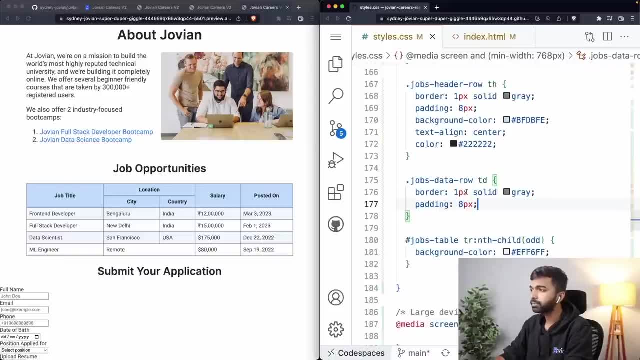 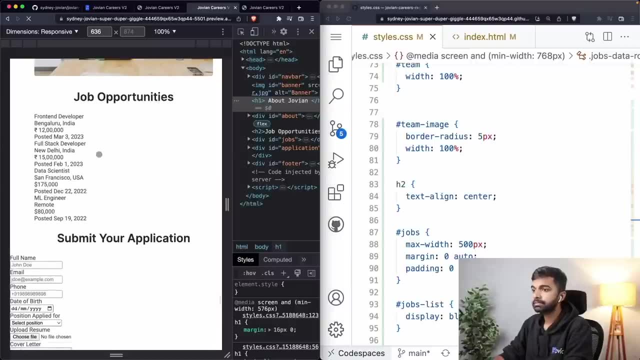 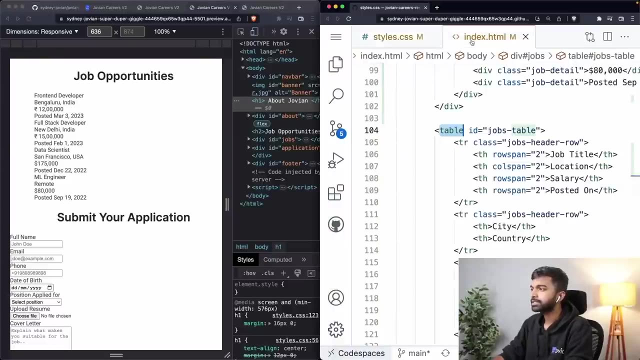 nth child. All of this is covered in the previous tutorial. Okay, All right, We're getting there, We're almost there. Now the only thing left for us to do is style this: actual job opportunities, this job opportunities div. Okay. 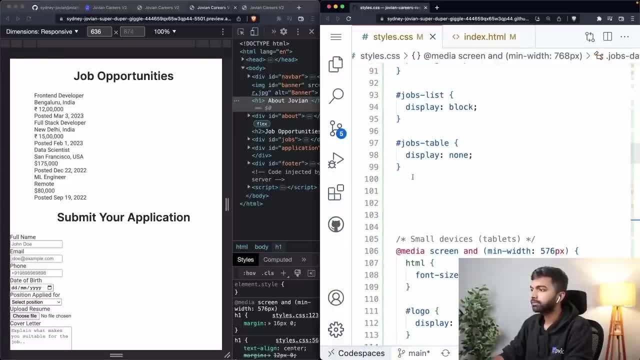 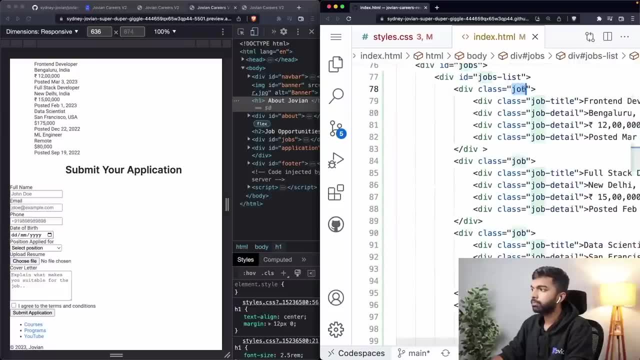 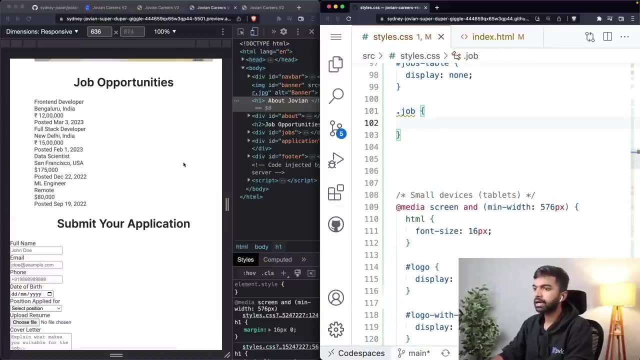 Let's try styling it quickly. So the job opportunities div is This: has each of these jobs as the class job. So first I'm going to style the job class for dot job And for the job class I am going to say: let's look at mobile. 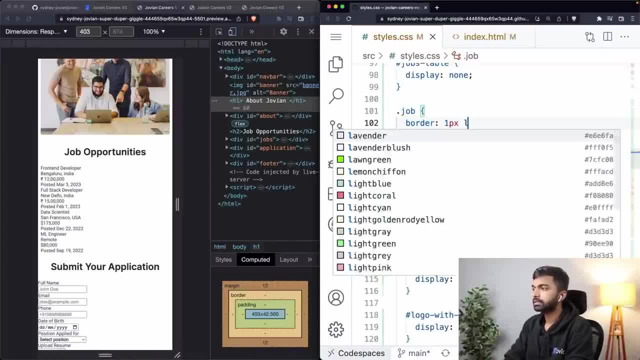 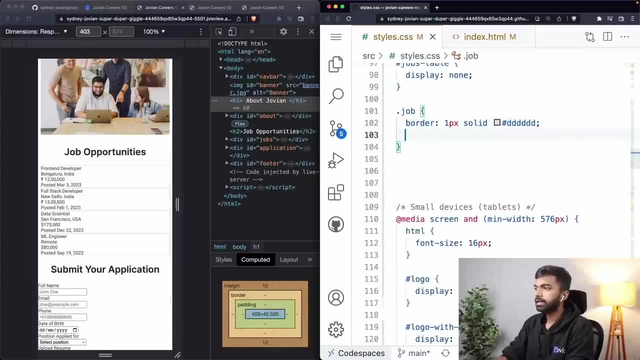 I'm going to first give it a border. a border, one PX, solid. I'm going to use a light gray, DDD, DDD. Okay, Now they have a border. Then I am going to give it a margin, top, margin, Top or PX, maybe even eight PX. 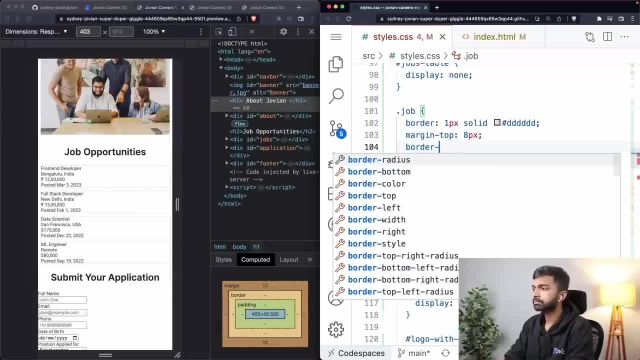 All right, I'm going to give it a border radius of five pixels. Okay, That's nice. Now I have a rounded border. I'm going to give it a padding of eight PX. Let's see what that does. Okay, That's looking good. 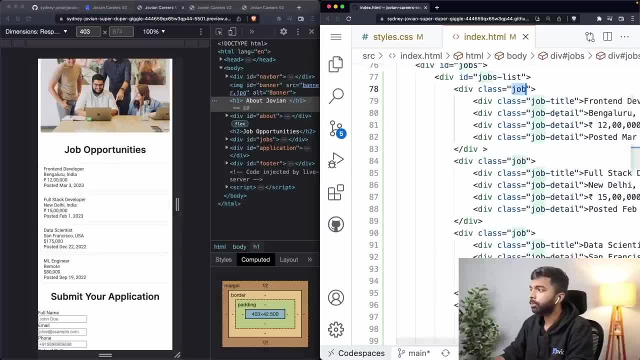 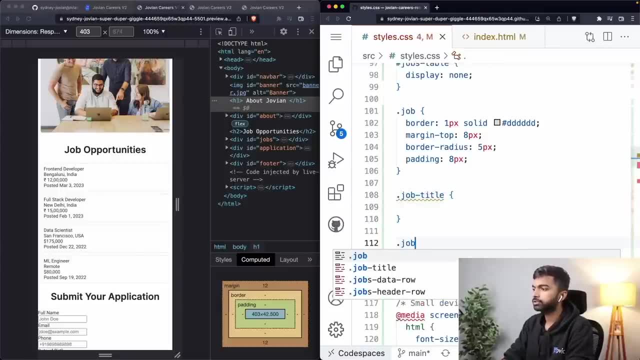 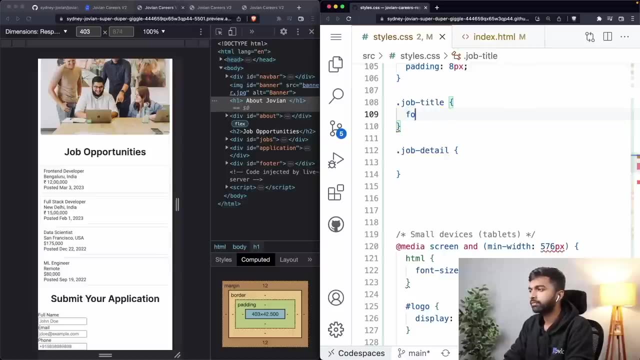 All right, So I have these boxes now, So these boxes are looking good. Then I have job title and job detail. Let me try and quickly style those as well. So job title and job detail. the job title is: let me see font size. 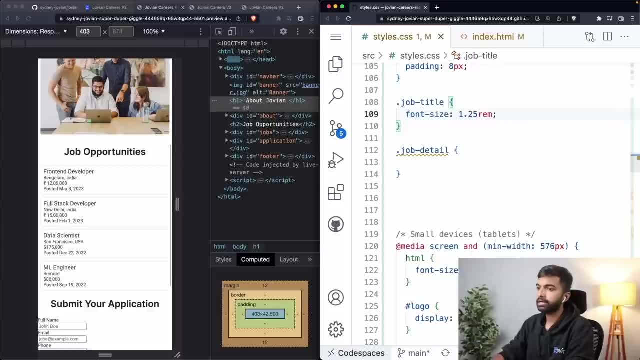 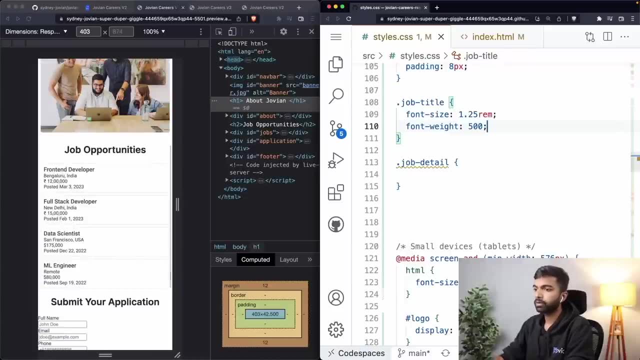 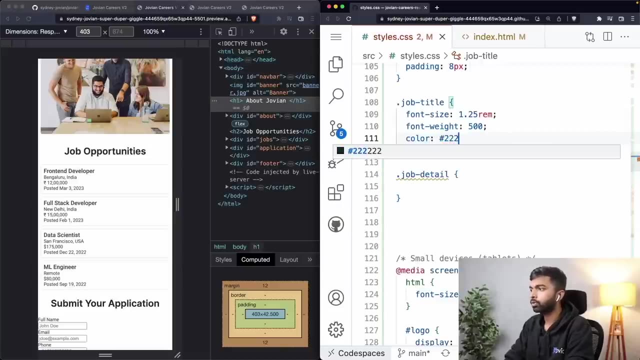 Let me give it a font size of 1.25 Ram that it scales accordingly. Let me give it a font weight of 500.. Okay, That's looking good. Let me give it a color of 22222.. Okay, That's good. 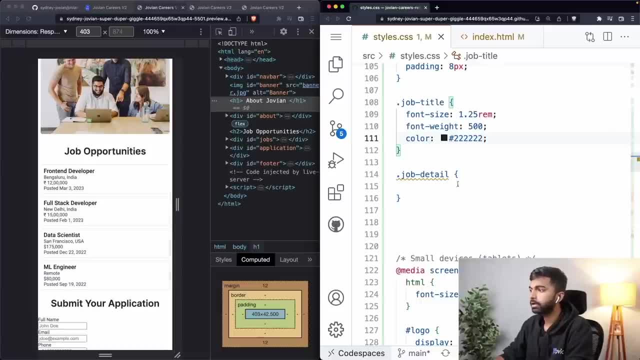 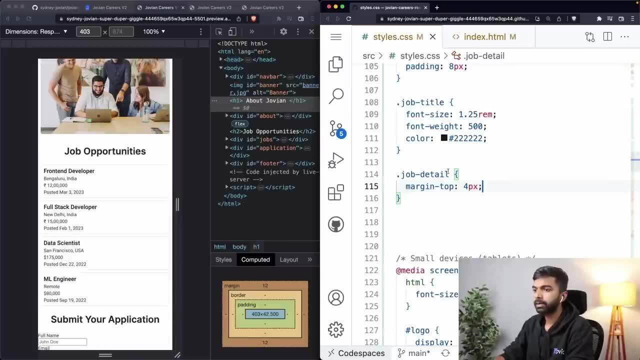 22222.. Okay, Color is looking good. And then for job detail, well, let me just give it a margin. top of four pixels is to space things out a little bit, And let me give a color of slightly lighter color. five, five, five, five, five. 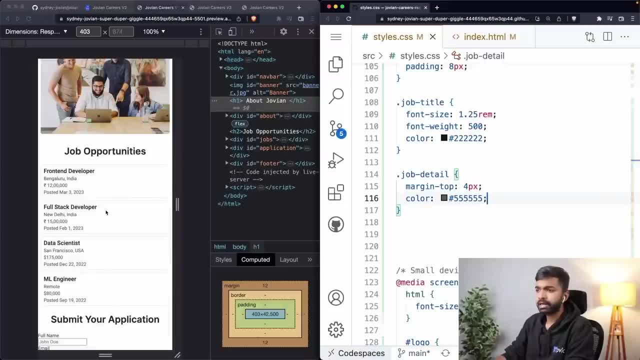 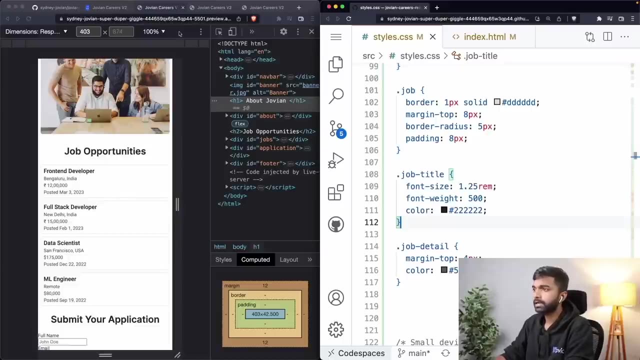 Okay, That's looking slightly lighter. Okay, I think that looks good. So I have some job. I have a border, I have this radius around it, I have this title. I have set up all of these details, I've put in some space here as well and I've given it some weight. 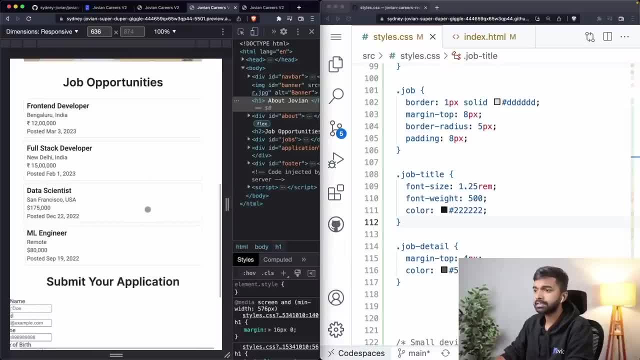 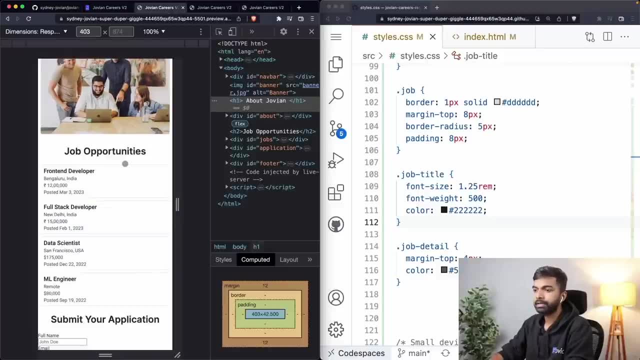 So that's looking pretty good. I think that's looking good on tablet as well, And it is centered on the page And that is looking that's just not visible on desktop. So with that we have completed the job opportunities section. 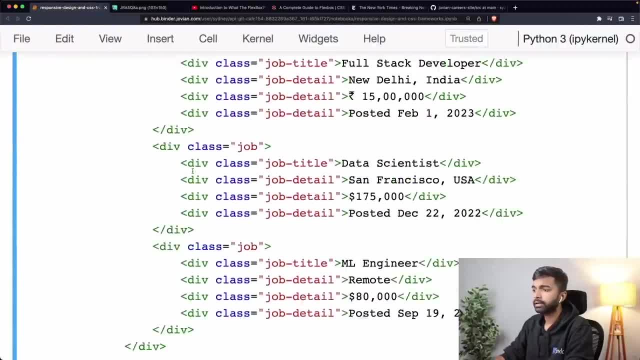 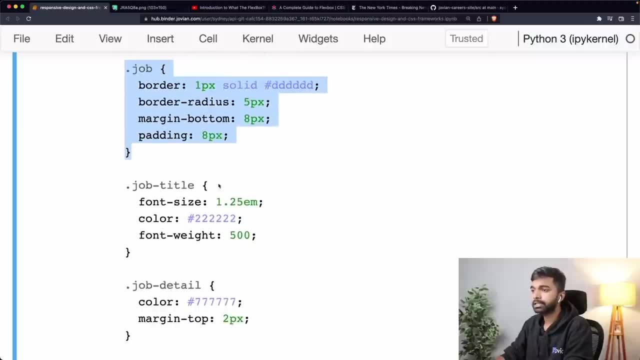 You can see, now we have the jobs list on mobile and tablet, And the way we did that was first setting a max width of 500.. Okay, And then for job: giving it a border, border radius, margin padding, a job title increasing. 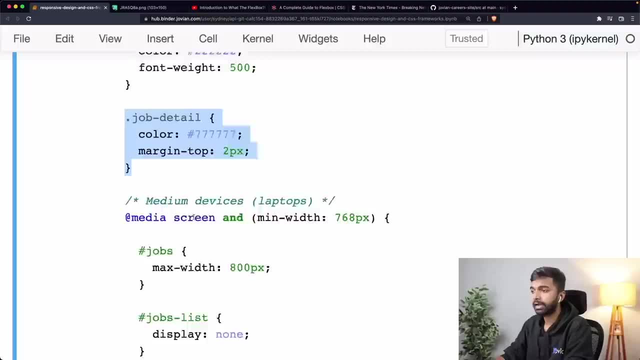 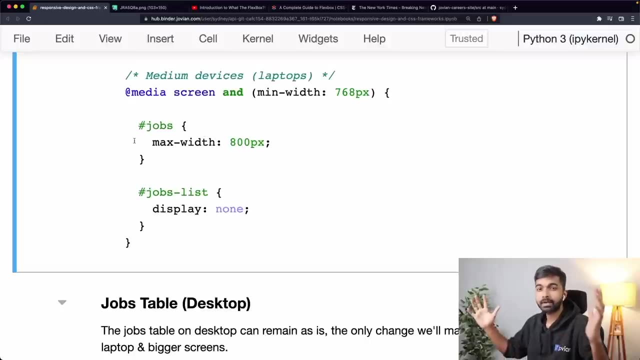 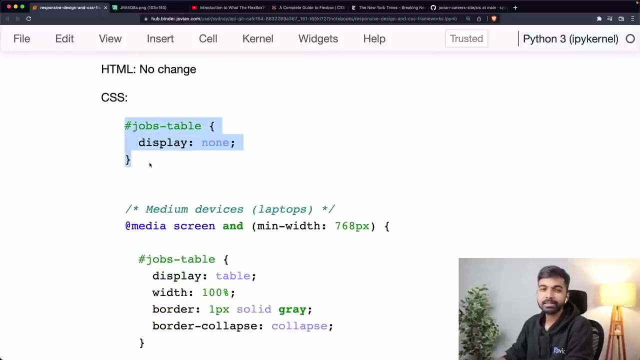 its font size for job detail increasing, making it lighter. And then, of course, on the min width of 768, we increase the max width of jobs So that it's a little bigger on desktop. And we set the job list display to none. for the jobs table on by default, we set its display. 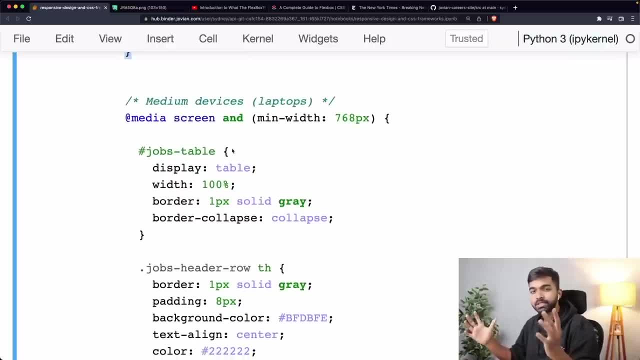 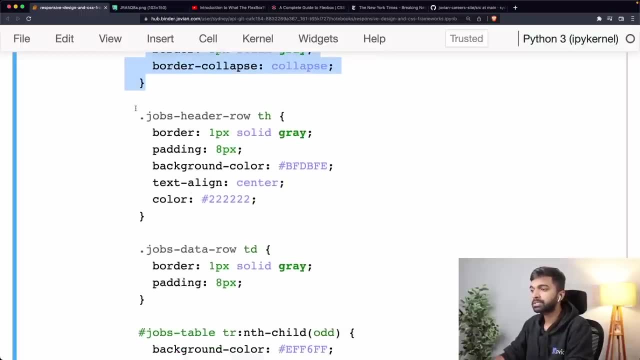 to none. And once we reach that 768 width when we want to display it, we set its display to table, We make it full width, we give it a border border collapse and we give all those settings which are required to show the table properly. 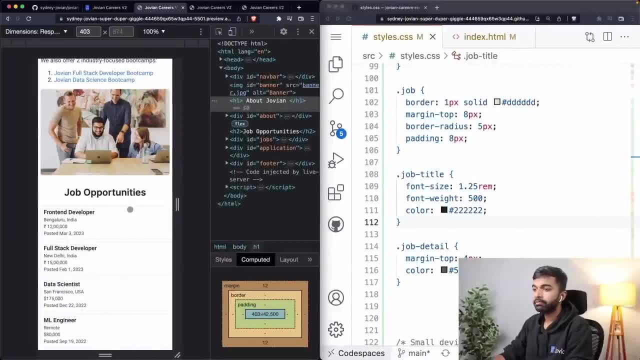 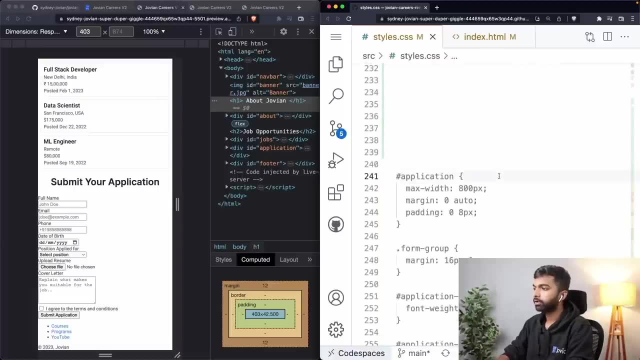 Okay, All right, We're on the last leg here. Let's go ahead and fix the application form as well. The first thing I'm going to do is just pull out all these application form settings right all the way to the top. 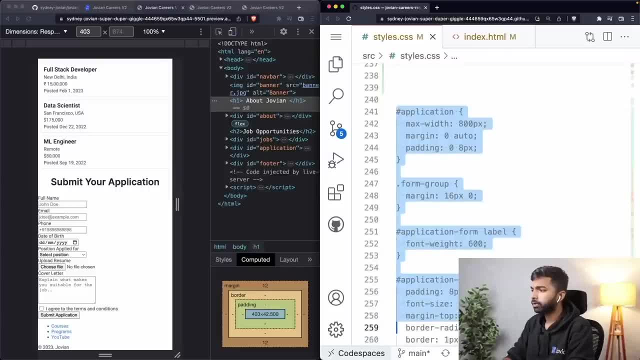 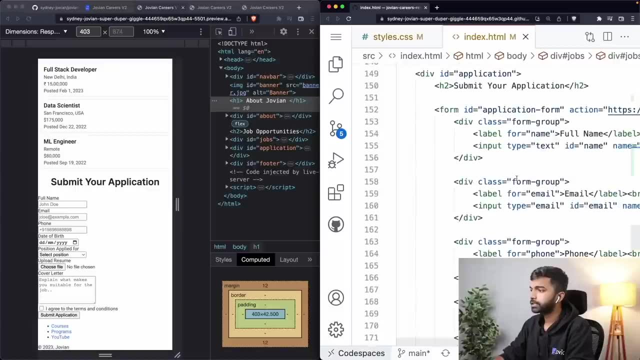 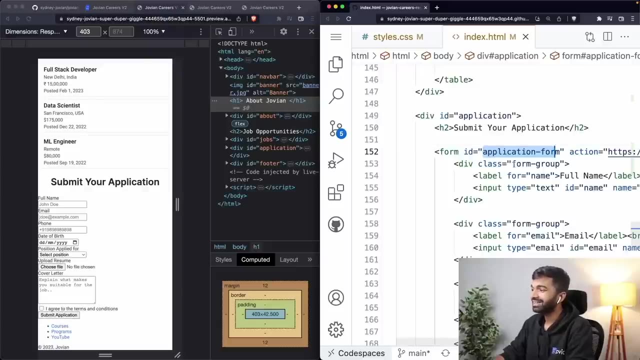 So let's see: have application form, group form, input, all of that Okay. So how it works is we have this application div And inside this application div we have an application form which is a form with the ID application form. then each of these inputs and labels are together part of a form group. 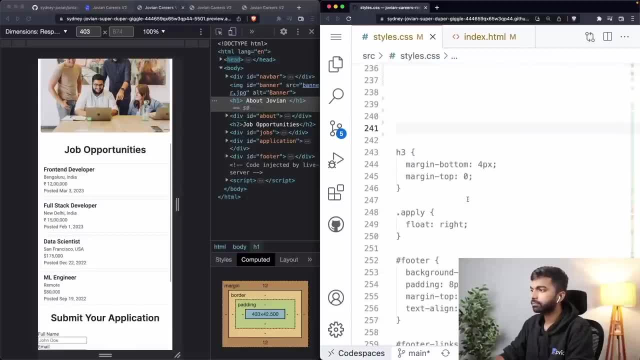 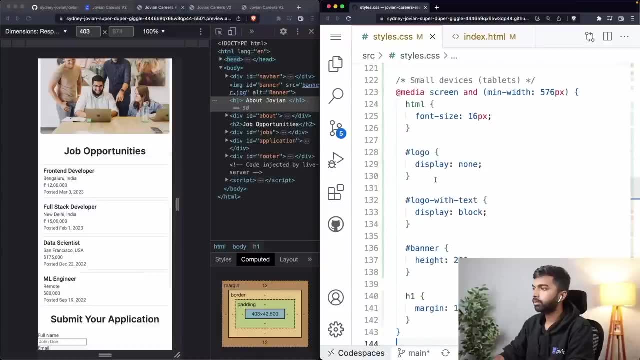 Okay, so we're going to use all these styles And we have a bunch of custom styles that we have set up for all of these. So let us go in and do that. Let's see, let's come in all the way to the top, above any media queries, let us paste. 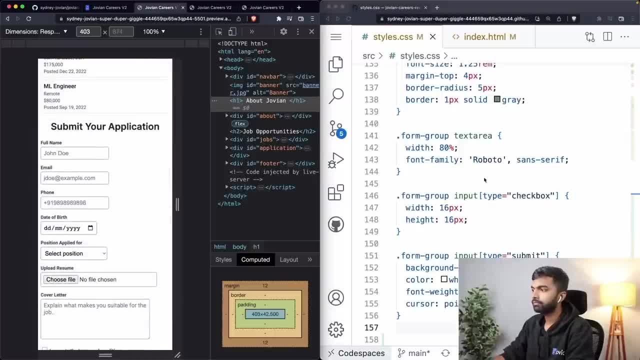 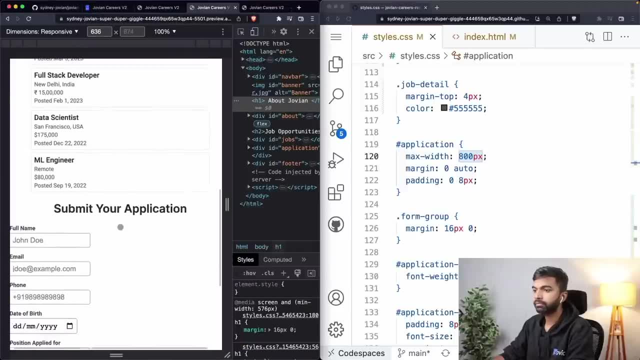 the styles, And this is what we end up with Now we have For the application itself, the max width is 500px- 800 pixels, So it takes up the full width, which is not what we want. Let's set the max width to 500 pixels instead. 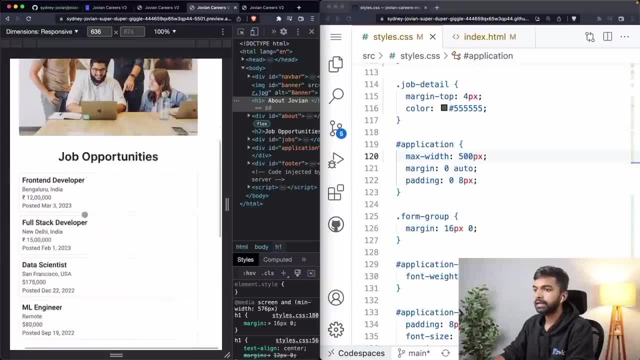 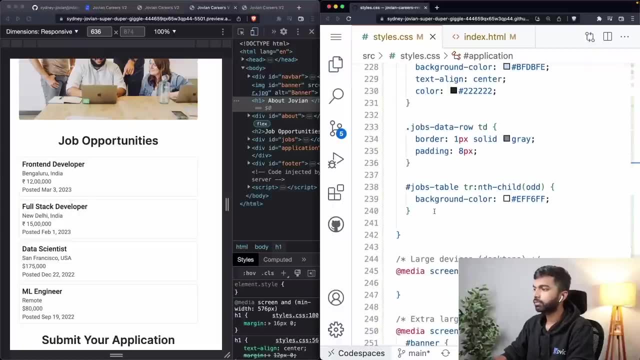 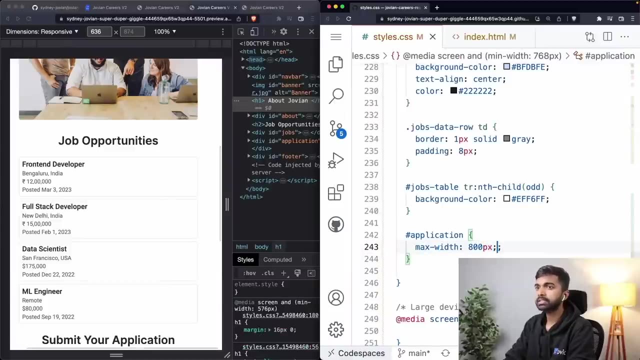 Okay, that's fine, And now it is in line. on tablet it is all centered, But of course we can go in and on the desktop version we can increase the max width, So we can say application max width to be 800 pixels. 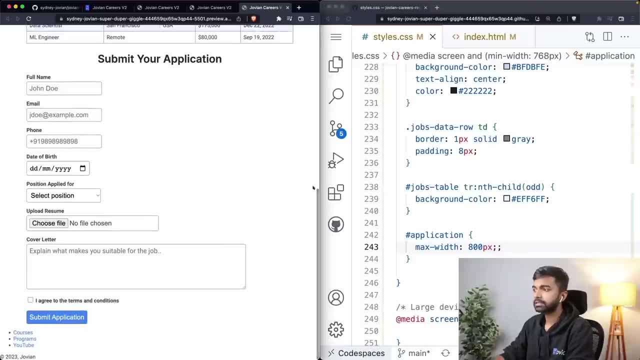 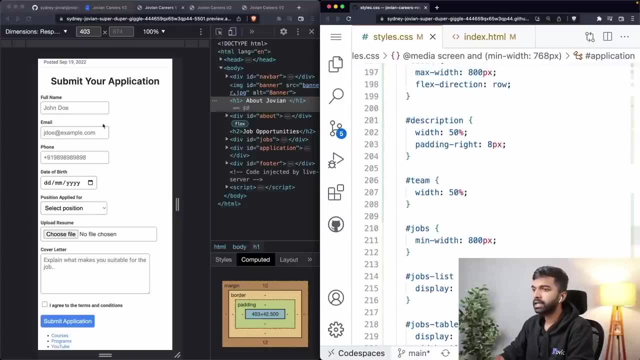 So that on desktop It still takes up the entire width. It's looking good. I think the only change I'm going to make here. it actually looks fine. The only change I want to make here is maybe make the inputs full width. 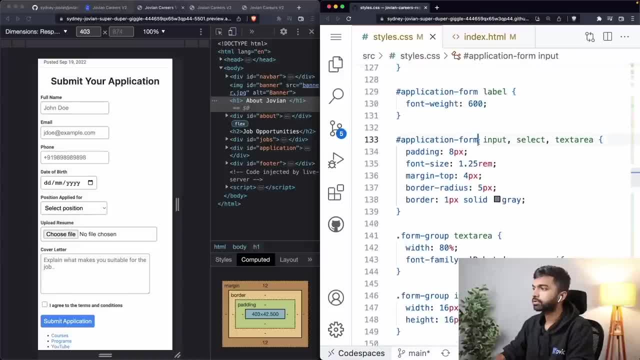 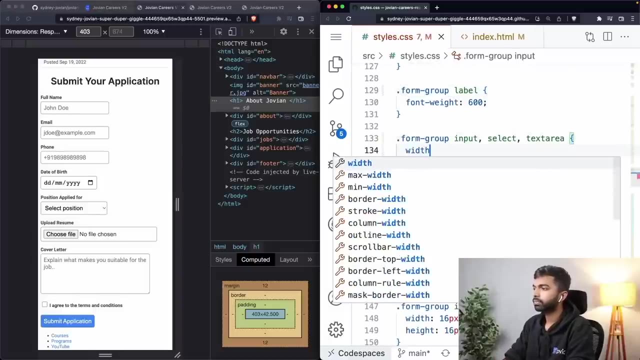 So I'm going to come in here, I'm going to change this to dot form group, because that is going to be more specific. In each form group, I want the label to have a certain. I want the input to have the width of of about 80%, let's say. 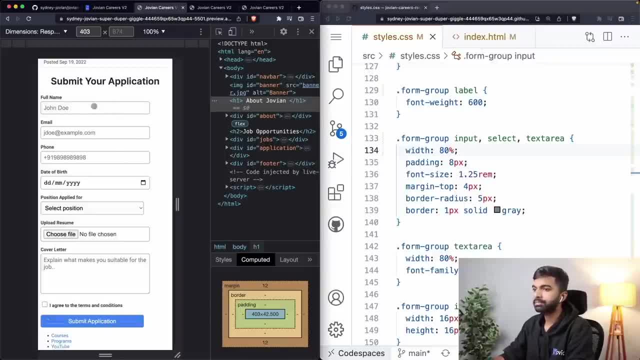 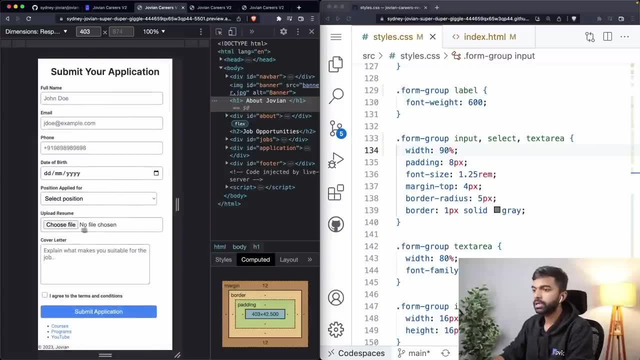 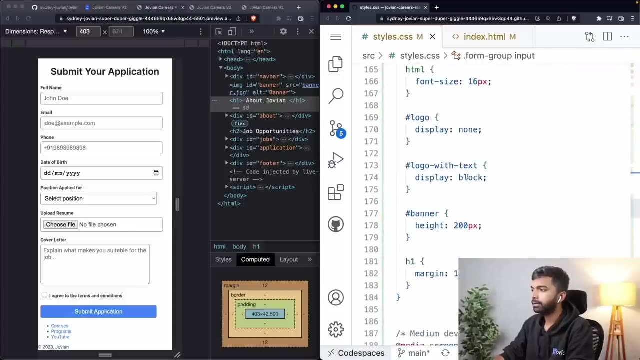 So that all the inputs are about 80% wide, something like that, maybe even 90%, just going very close to full width. Yeah, So I want all my inputs to be about 90% wide on mobile, But as soon as I get to the tablet, on tablet, I don't want it to be 90% wide. 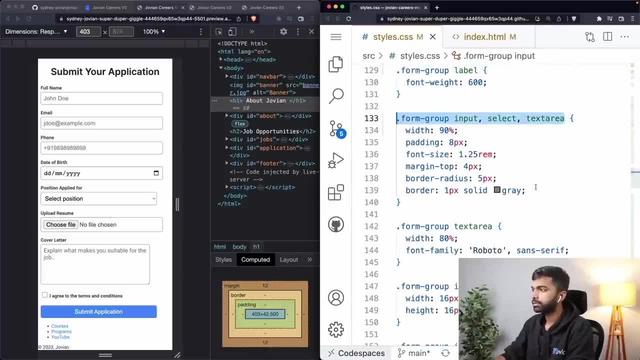 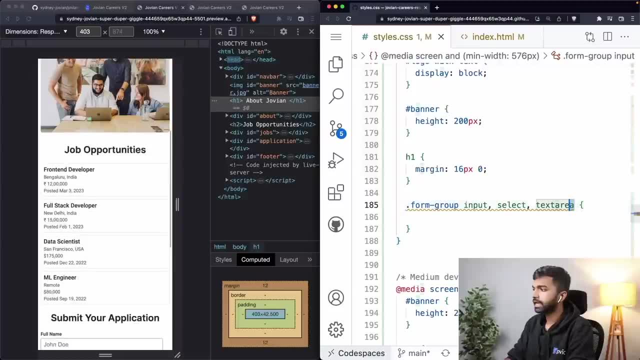 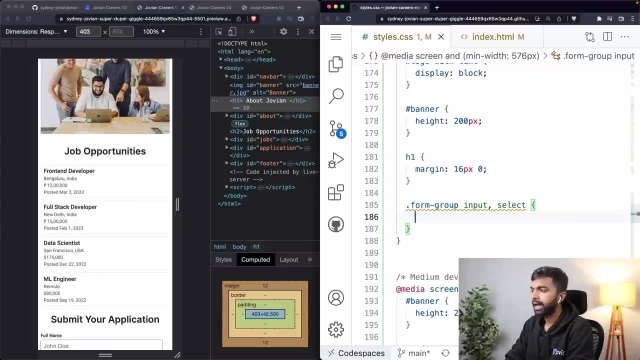 So I'm just going to go in here on tablet. I'm just going to set 90% Input select text area. it doesn't need to be modified. I'm just going to set max width or width to be about to be auto. 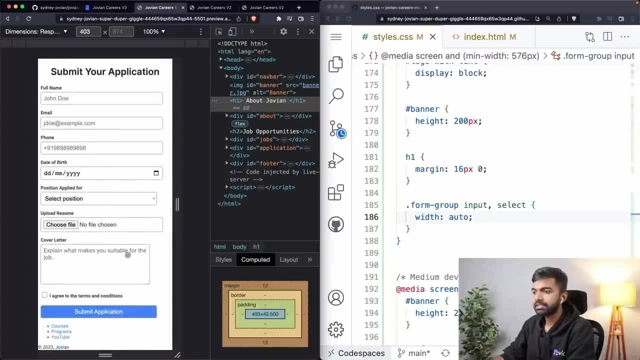 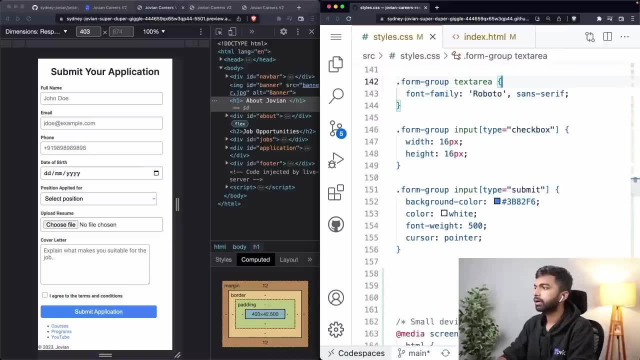 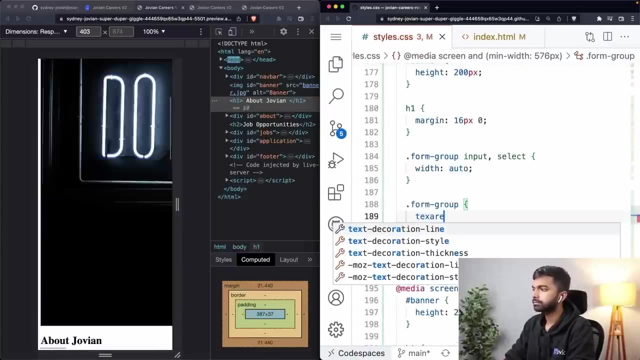 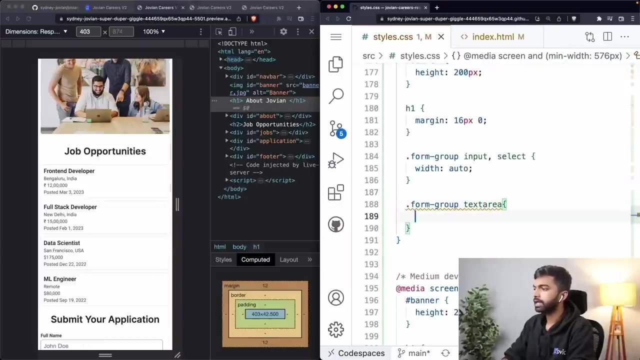 So on mobile it takes up about the full width And that's nice, And on I can remove this with 80% here and set that manually here. So dot form group: text area for text area. we still want it to be a bit wide, about 80%. 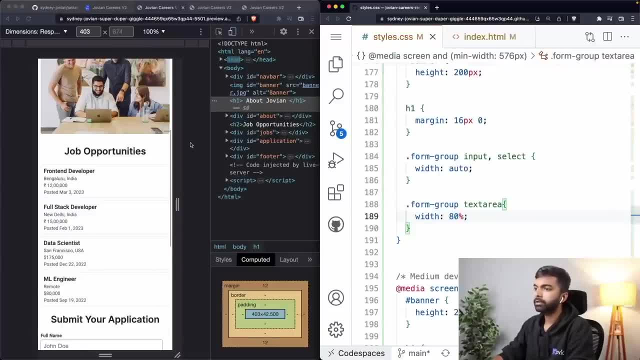 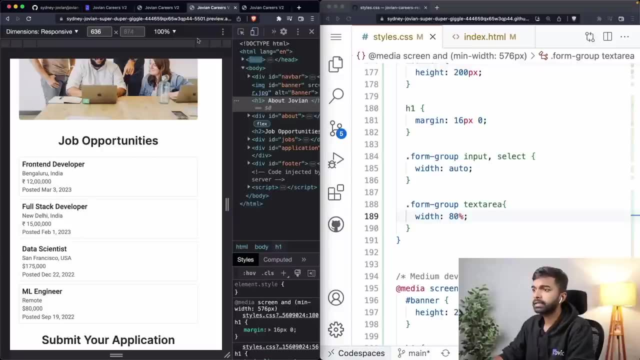 wide, or even on tablet. on tablet, what this is what it looks like. the application look on. the application on mobile looks like this: almost full width. the application on tablet looks like this: So it is not taking up the full width, but it is still centered on the. 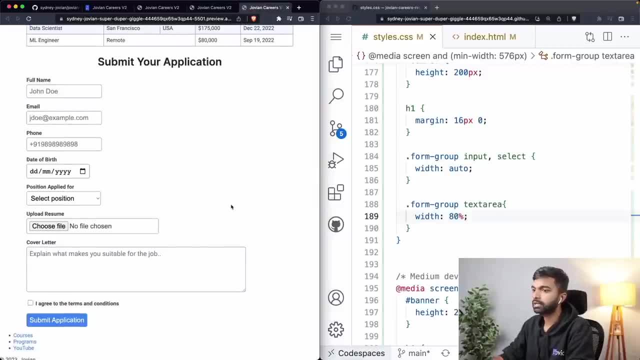 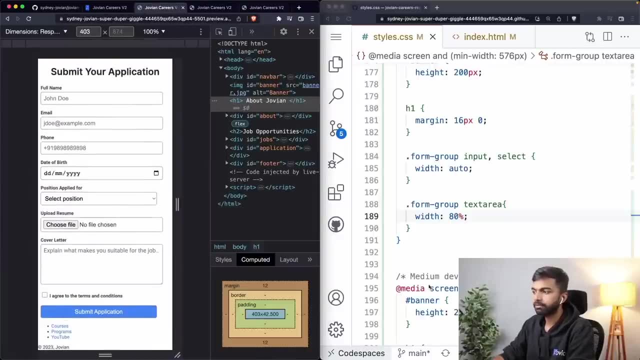 page, along with the rest of the content and the application on desktop looks like it used to. There's no change there. Okay, so that's nice. The final thing we need to do is fix the footer, So we have a footer right at the bottom. 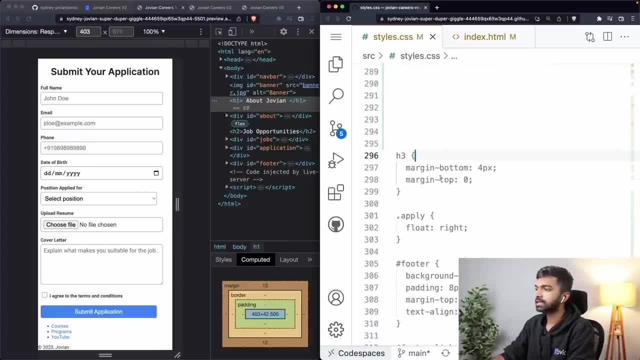 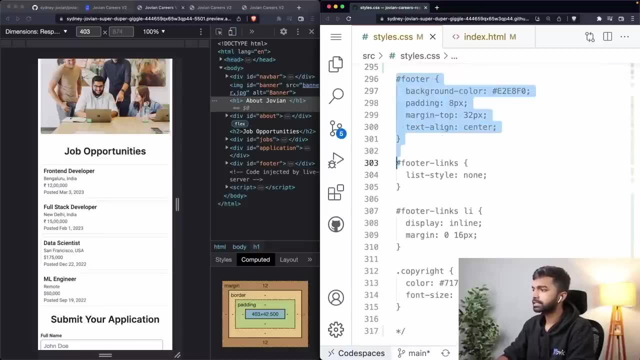 Let's go ahead and fix the footer. The first thing we'll do is just copy over all the existing styles. We don't need this h3,. we don't need this apply. I'll get that. we just have footer, footer links, footer links, Li and copyright. be that. with that, we've exhausted all the style. 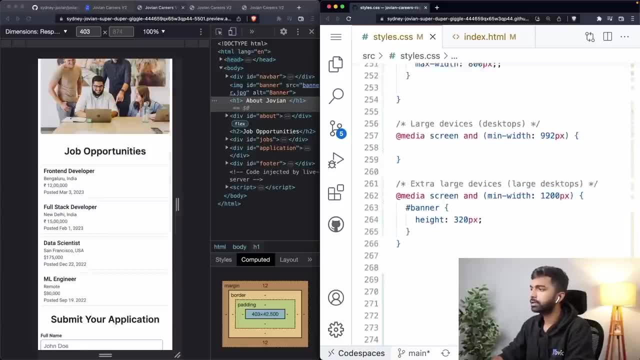 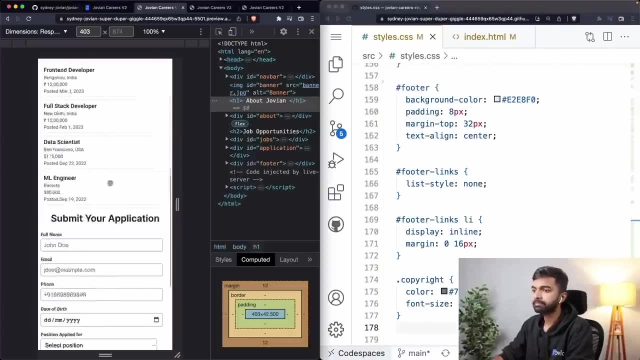 Yeah, So we've carried over all the styles, So let me just go in right at the top. before we create any media queries, Let's put in the footer styles. Let's see what that gives us. Now we have a footer which has this background that we're looking for. 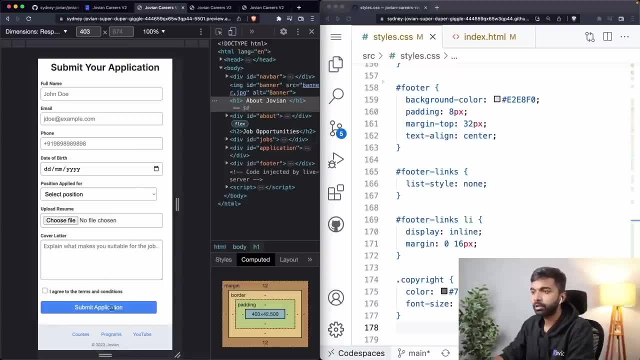 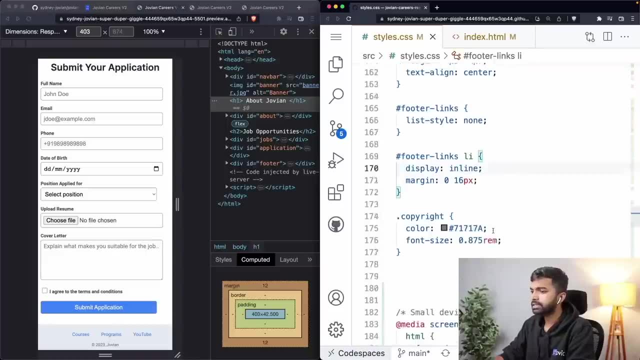 And it has these links And it has this copyright. all of that is good, But on the mobile, we want these links to show up one below the other. And how do we do that? Well, you see, we have this display in line for Li. I think we can get rid of this. 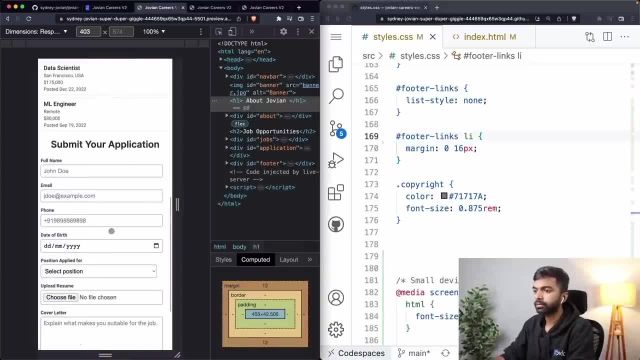 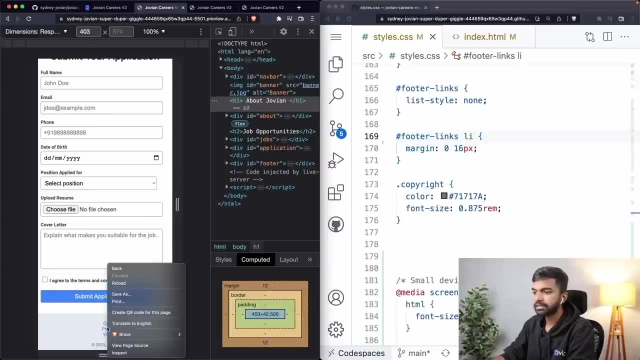 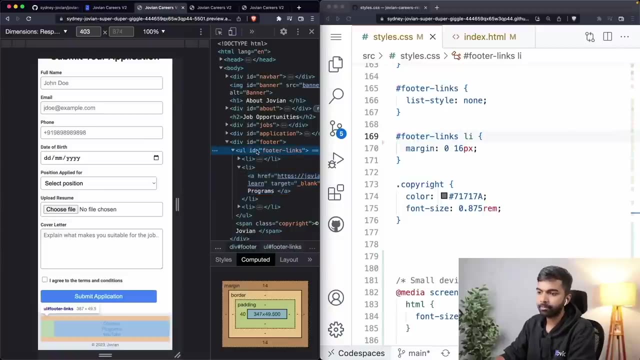 Okay, So we're going to show up one below the other. Okay, And it looks like they're centered now, but they're slightly off center. So if I just inspect this list, I can figure out why it is off center. All of this seems to be centered, but it looks like this ul, this unordered list, seems to. 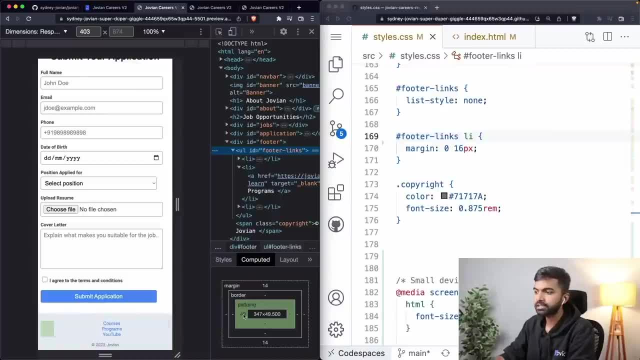 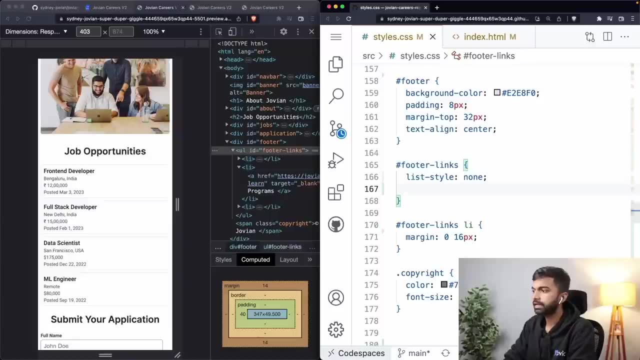 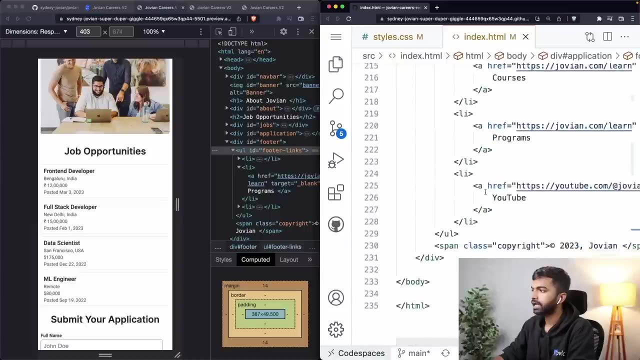 have a padding on the left, you see that green color thing. that is just this padding on the left. Let's go into the footer links list and let us just set padding Okay, Left Zero, Right. So that's what we have here. we have this footer. if we have the footer links, ul and. 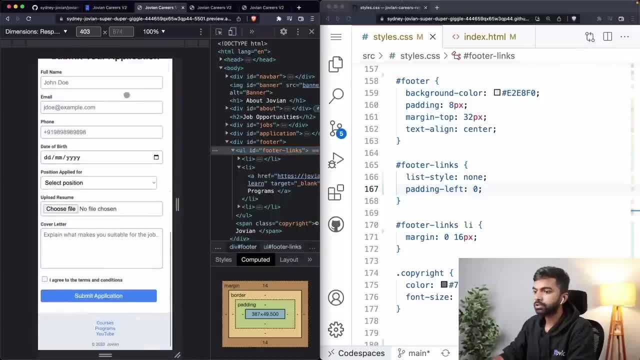 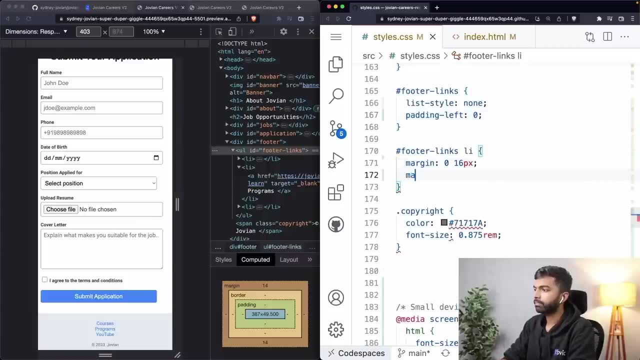 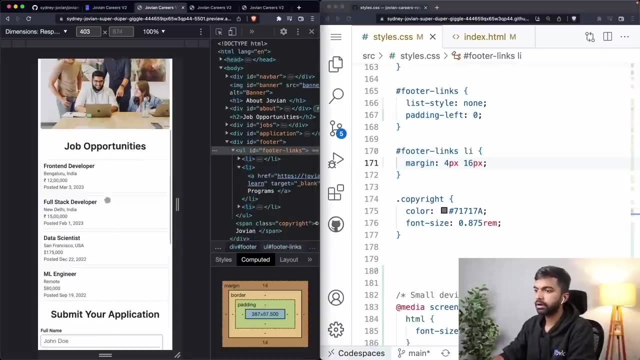 then we have a bunch of allies And that is now doing the footer, the footer items, one below the other. I may even add some margin bottom So I can say margin or px and 16 px. So now I have a margin bottom so that they're slightly spaced. 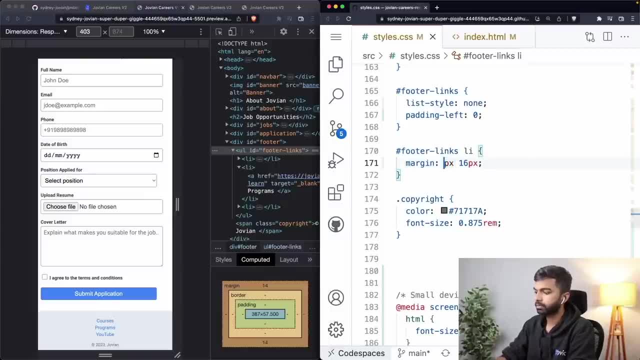 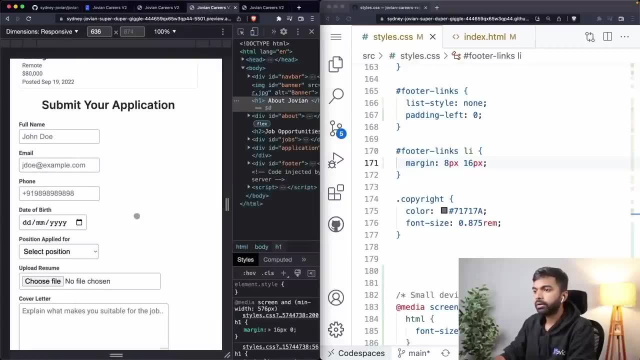 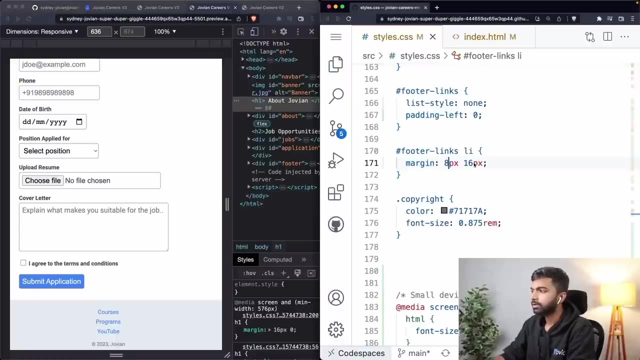 They're slightly spaced out, maybe even 8px. Okay, so this footer is looking nice. Okay, let's see on tablet. Now, on tablet, this footer is probably not looking good. I think I can just get it back to inline. 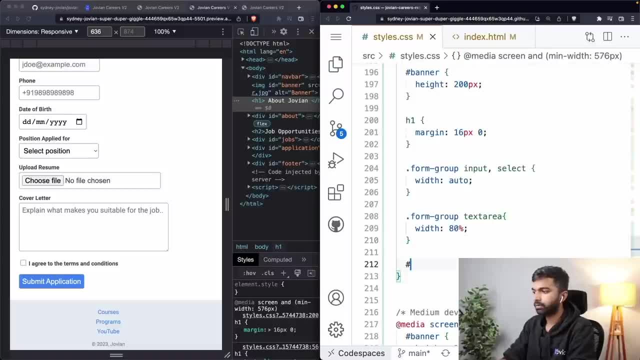 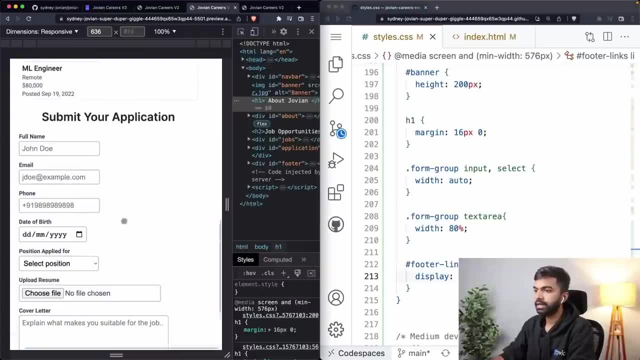 On tablets, I'm just going to come in here And I'm going to say footer links, li, display line And let's see. Okay, so on tablets, it is inline. On mobile, it is still one below the other. 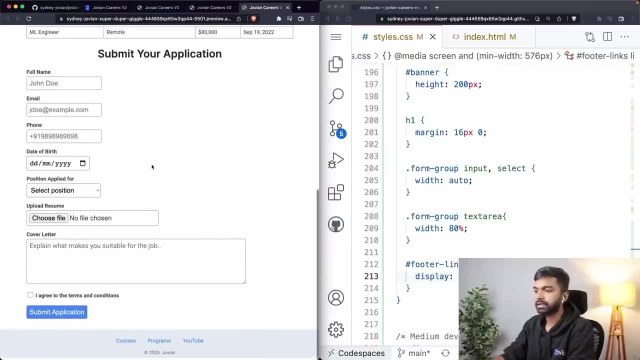 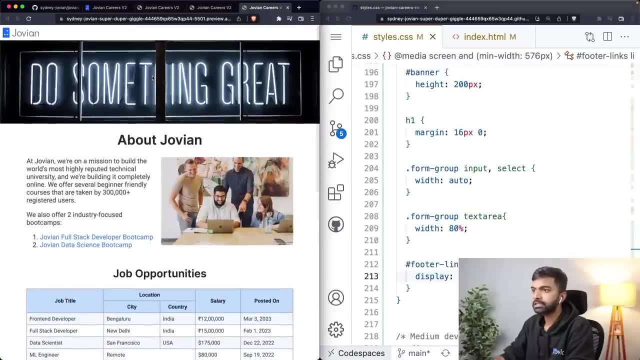 This is what I'm expecting And on desktop it is inline Perfect With that. we have completed the footer, So we've done the. we've done all the sections. I think all of them look good on mobile, tablet and desktop. 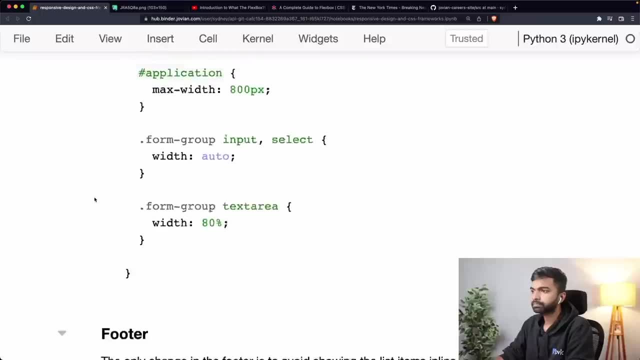 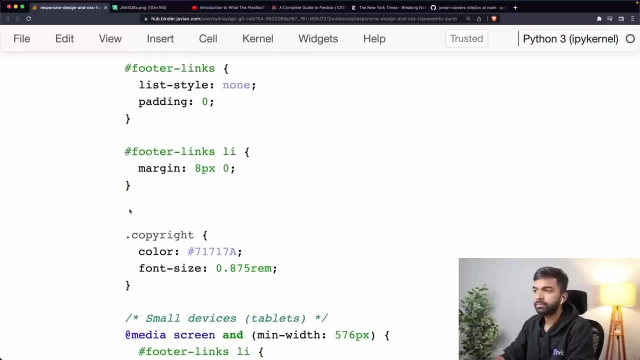 That's good. We have done the changes to the application form. The only changes we made was some width adjustments for the inputs And we have done the changes For the footer. the only change we made was that we wanted to show them one below the. 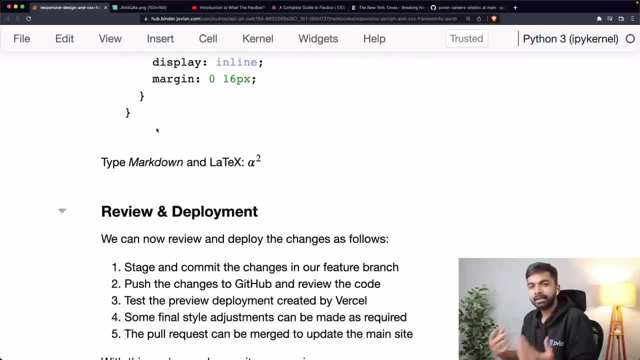 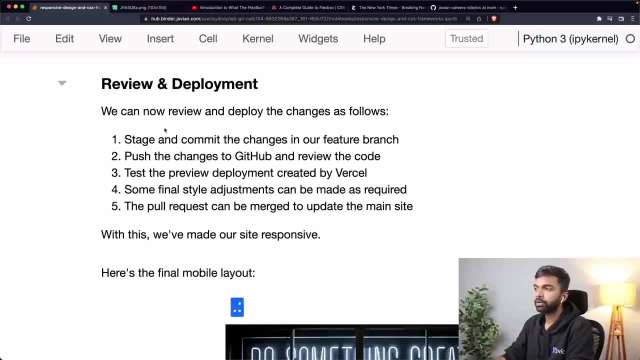 other on mobile and side by side on desktop, and again practice this, work it out step by step. That is how all of these steps will make sense. We can now review and deploy these changes. So what we're going to do is: first, we're going to create a branch, is going to do that here. 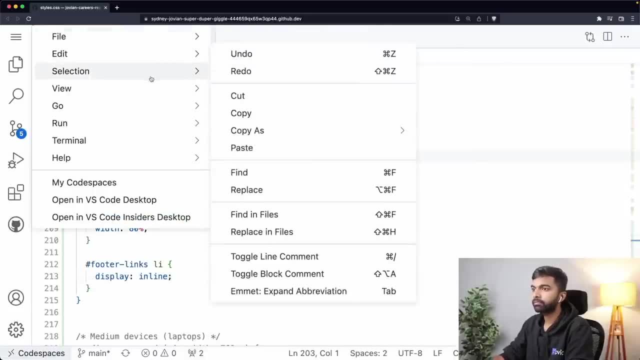 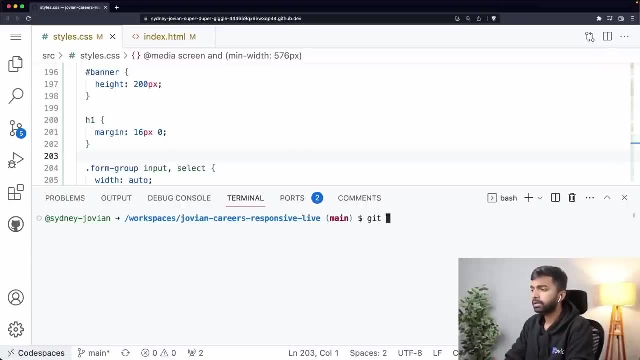 by first opening the terminal. So let's say: if I do terminal, I'm going to first create a branch. Let's do git checkout. Okay, I just be minus. B is a quick shortcut to create and check out a branch in one step. 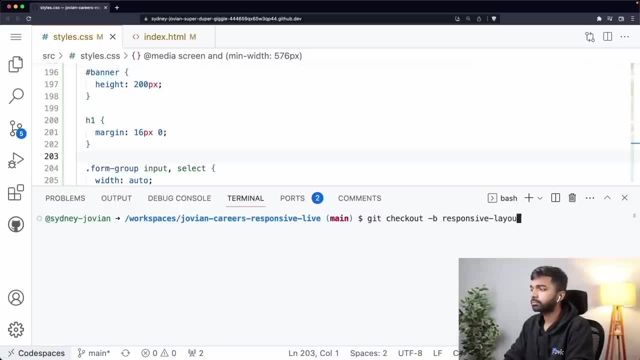 And let me just call it responsive layout. Okay, now we've switched to a new branch. we've created a new branch and switch to it. You see, we are on the branch responsive layout and I'm going to do git, add dot. I'm going. 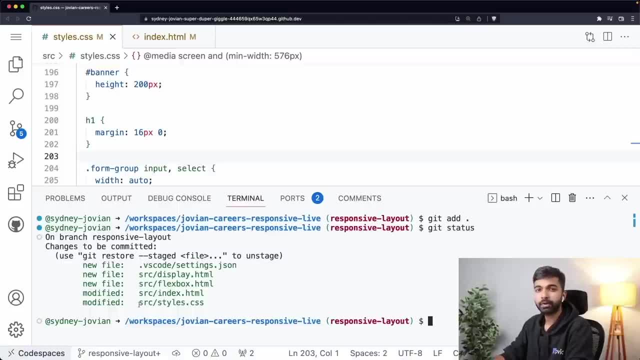 to review the changes using git status, you can see that a bunch of new files have been added. There's a settings or JSON as well, Not sure what, that's what, but it's okay. Then I'm going to do git add. okay, I'm just going to do git commit minus m added responsive. 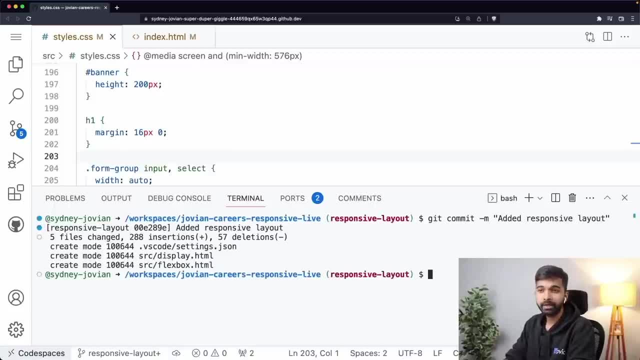 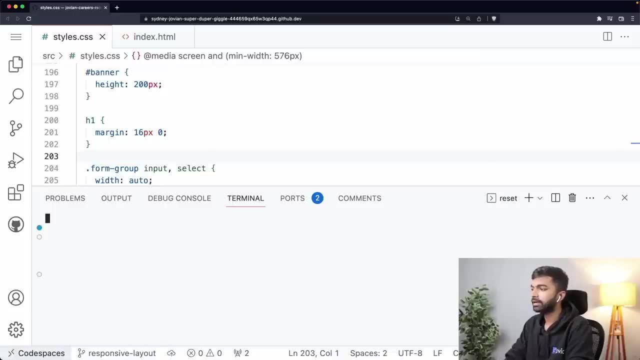 layout. Now we've committed it. normally I would commit after every section and keep updating my pull request, But just for now, just for example doing that, then let me do git push: origin responsive layout. Okay, So we stage the changes using git add. we then commit the changes using git commit. 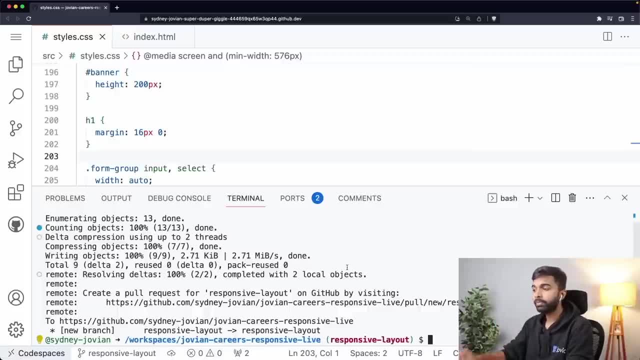 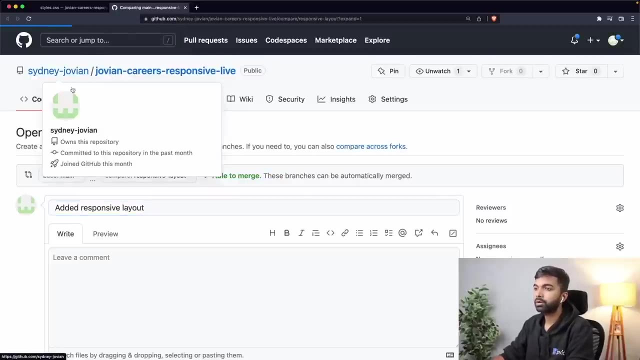 and then we create a push that branch to GitHub using git push origin branch name. Okay, Now we can create a pull request. So there's actually a helpful, there's actually a helpful link here that that is printed out for us, But we could always just go on the repository page. 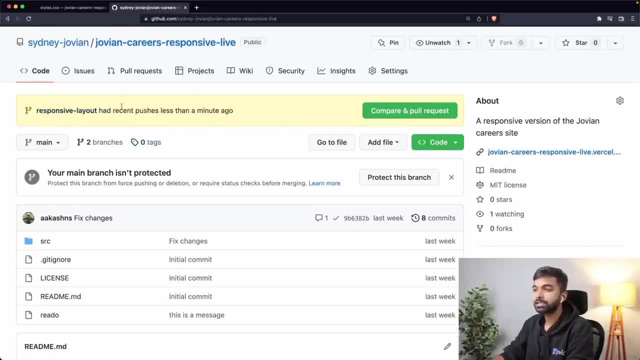 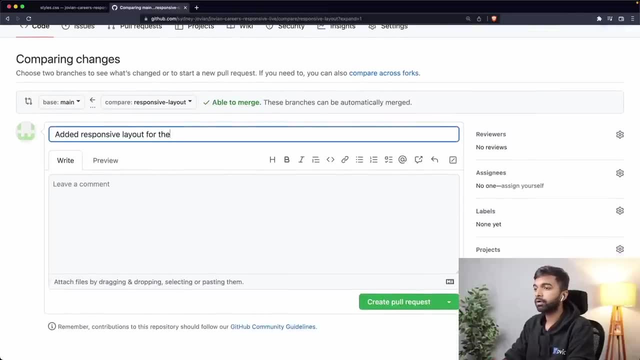 And on the repository page you can see that GitHub tells us that a responsive layout branch has just been pushed and we can create a pull request. So here's what we can do. We can see that, Let's say, I did a responsive layout for the jobs page. 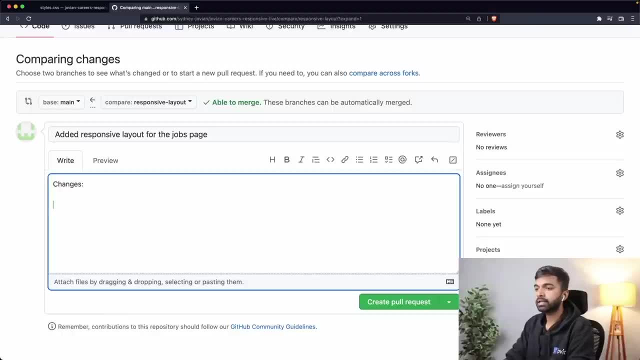 And I can mention changes And I can just bring in the changes that I've made here. So let's see, Navbar has a logo without text, Then banner size is updated Based on screen. Okay, Then about section is vertical first, then horizontal. 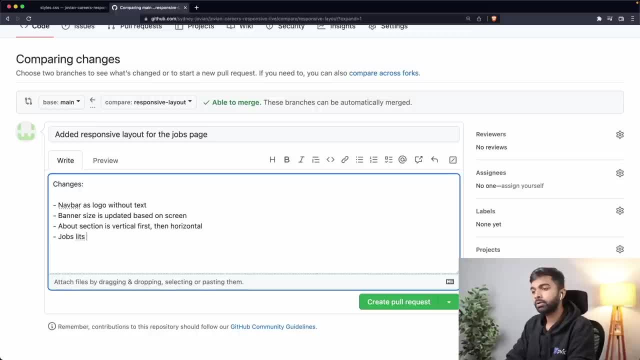 And then we have the jobs list on mobile and tablet And table on desktop. What else? Application form full width inputs on mobile: Okay, Let's see What else. Attachments Adds inputs on mobile And vertical Order items on mobile: okay. 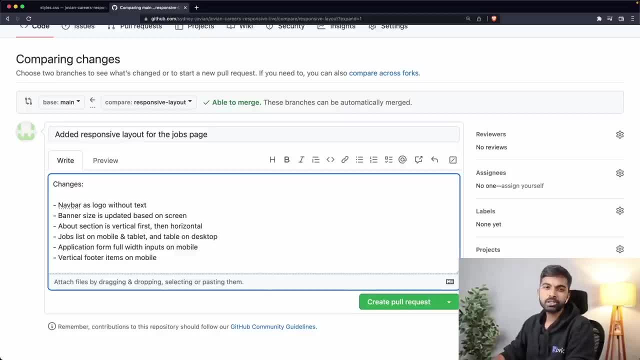 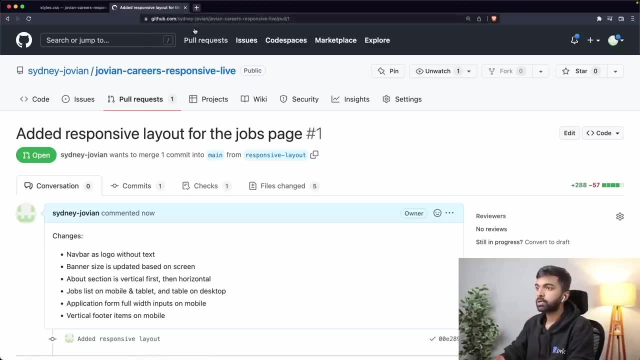 This is a short description of the changes and we can create this pull request And now you can see that our joven careers responsive site, which is our initial website. So in careers responses: dot for sale, dot app live- What's there? 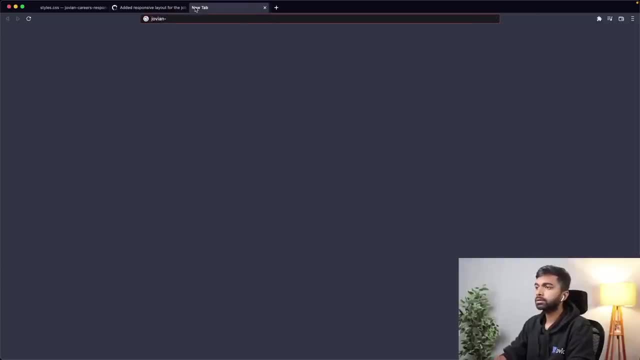 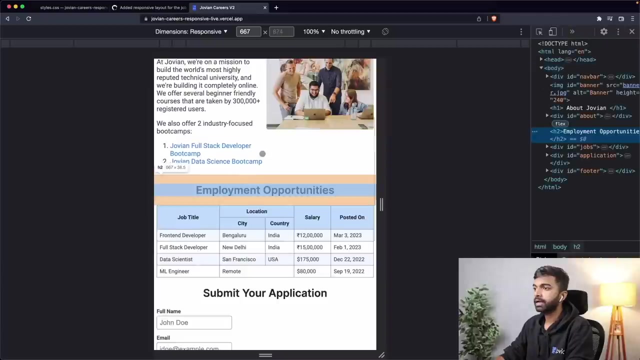 So in here we have our job list And this is our job list And you can see that our job list is here. And then our job list is here. This is still not updated. This still has the old design. In fact, I can go in and to inspect. I can verify this, that it's still trying to show. 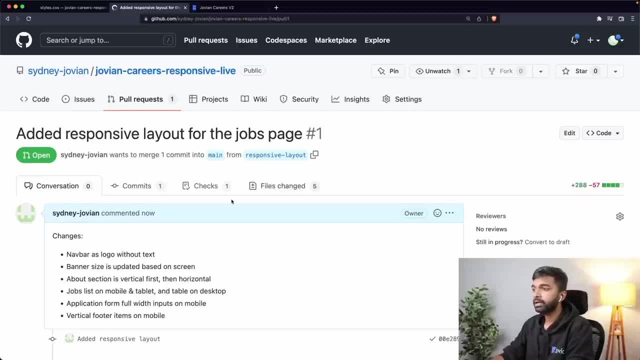 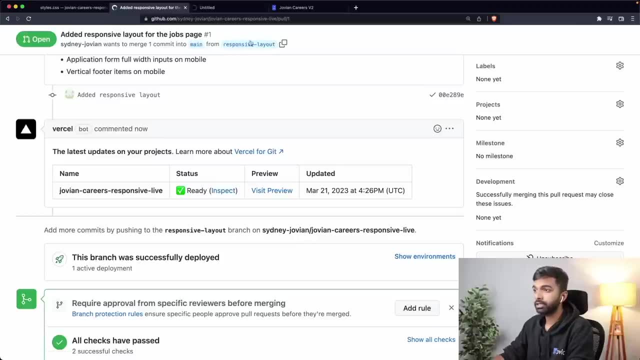 the table is trying to show things side by side, But now you can see that in this particular pull request, Vercel has created a preview deployment so I can visit this preview deployment. This is just for this branch And you can see that on this preview deployment. 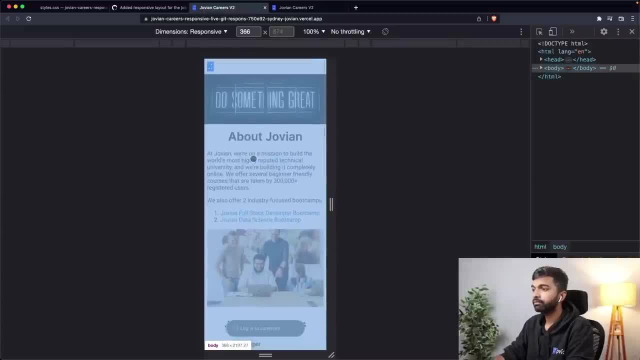 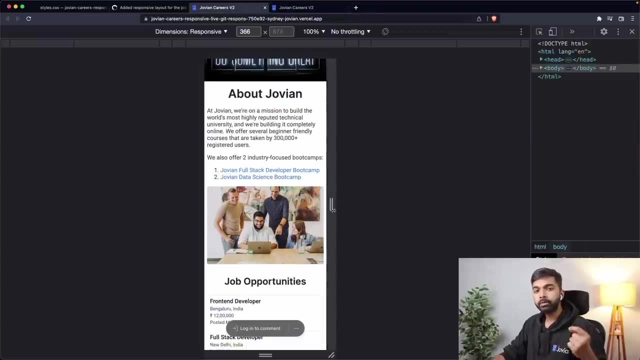 If I go inspect, we have our new layout. This is what you want to do. your main website is, as is, no changes there, But on your pull request you've made all these changes on your branch and you can test it out. So somebody who is looking at your branch can first look at the preview deployment and 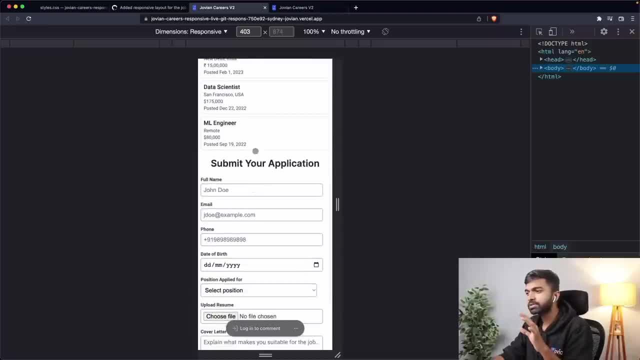 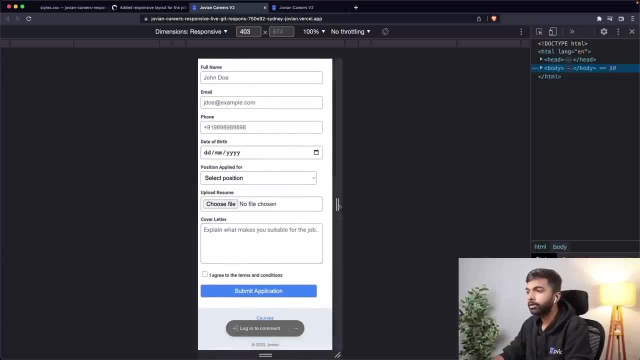 that maybe the designer can take a look and tell you: okay, maybe you need more space about submit application. Maybe there is some change to be done in job opportunities. Maybe the footer is not looking nice. Let me rework that a little bit. 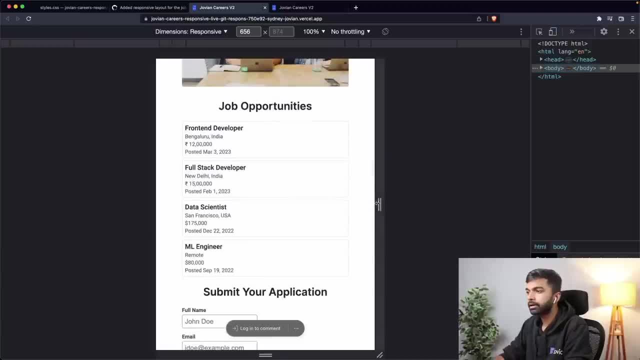 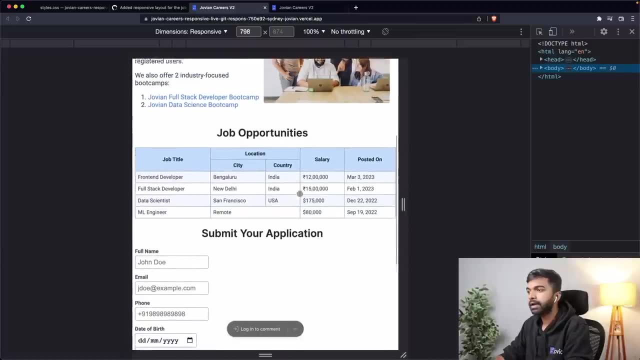 You can also maybe just see how things change. You can see that, okay, job opportunities takes up the full space. then it takes to around 500 pixels, then it suddenly expands. And now, when it expands, here you get this two column layout and here you get this table. 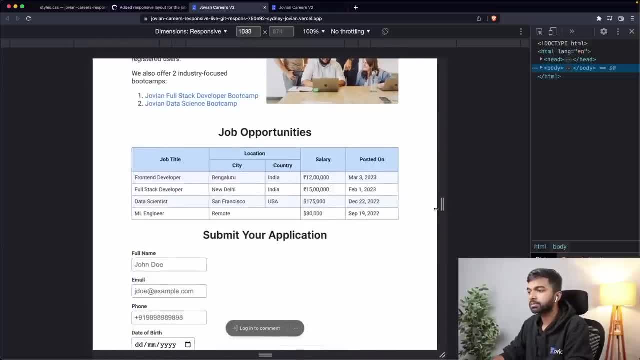 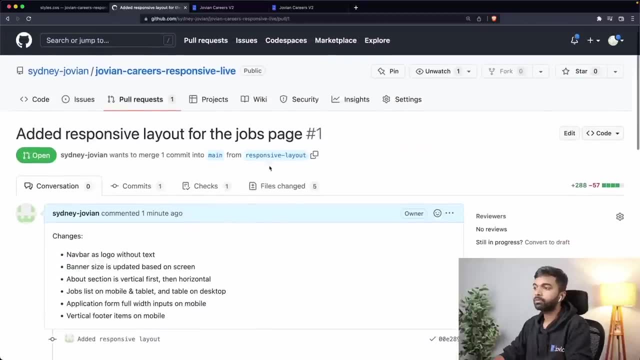 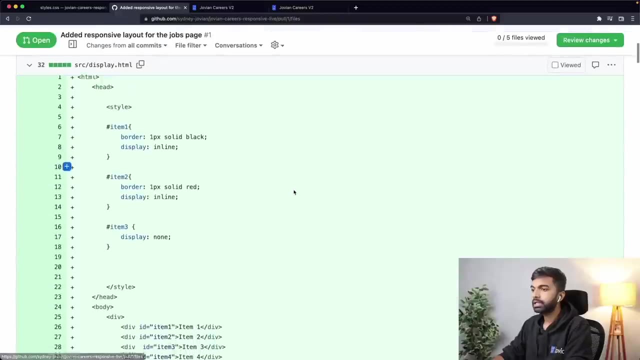 And that is looking rather nice And the application also expands accordingly. So the designer or maybe another developer can review the changes visually by looking at the preview. They can also review the changes manually, so they can go in and they can actually check it. 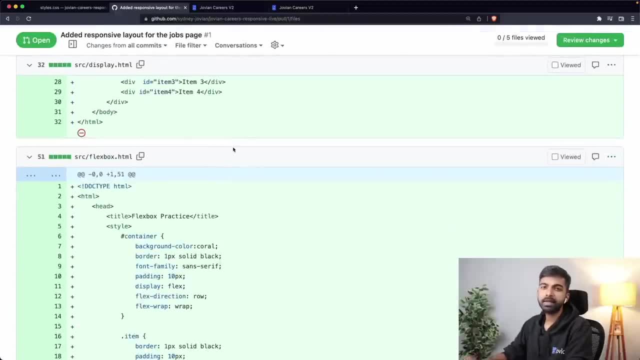 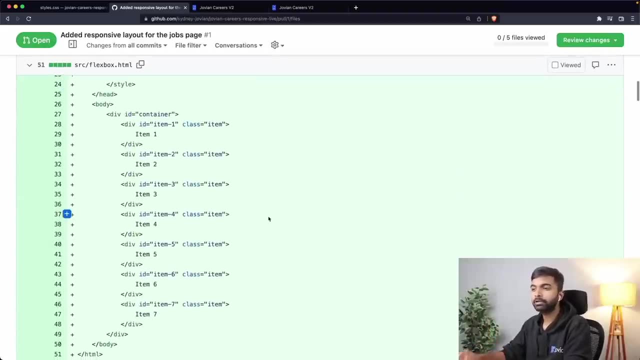 In each section. Okay, looks like we've added a display or HTML file. they can tell you. maybe we don't need this display or HTML file. get rid of it. We don't need this flexbox or HTML file. So you can go and delete those files and update your pull request. 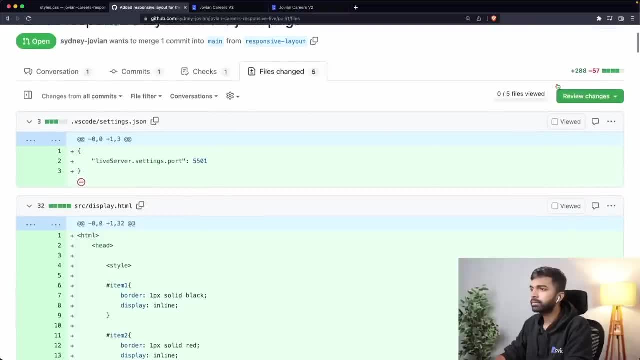 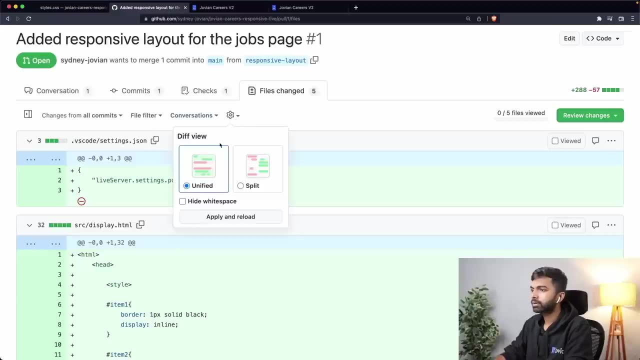 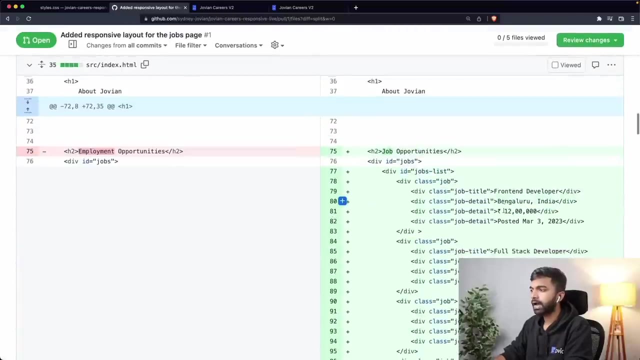 And okay, they can see. see a splits. So there's a split view available as well. Let me just hit view. Yeah, you can see a split view. Yeah, So you can see here The changes that have been made, that you have added this jobs list, as expected. 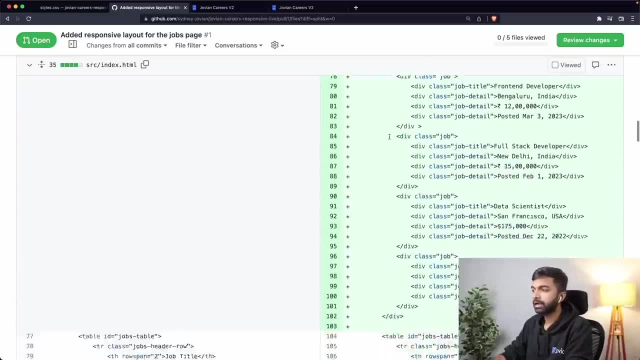 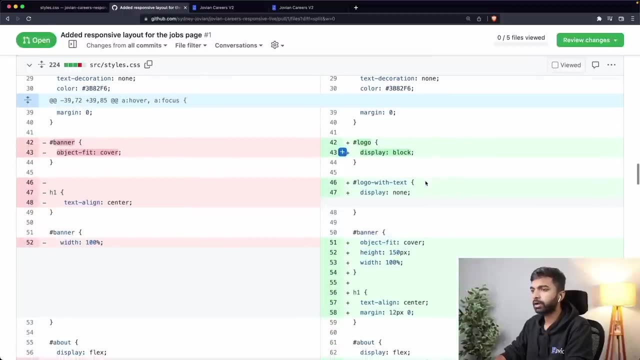 And you've not modified any other HTML except adding the job list and changing the title here. They can see here that you've added a bunch of base styles for mobile and you made it 14 pixels. you've not changed a lot else, maybe a few things here and there. 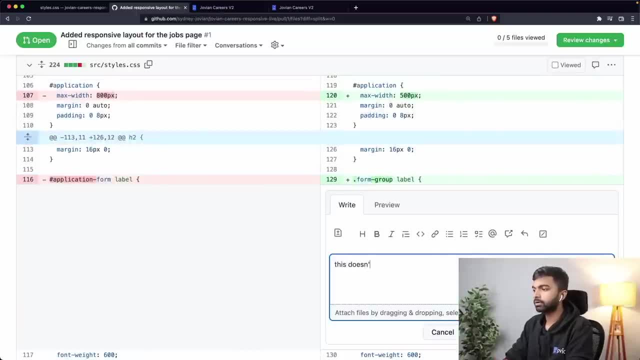 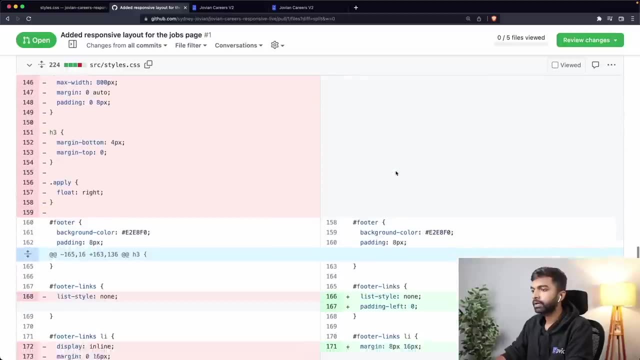 And they can give you inputs on specific things they can give. okay, this doesn't look right And they can comment it, and then you can revise those comments and pull your branch again and so on, And they can see that. okay, now you've added a bunch of these media screen settings and 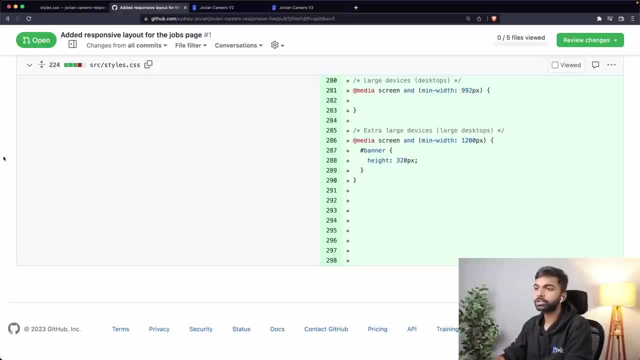 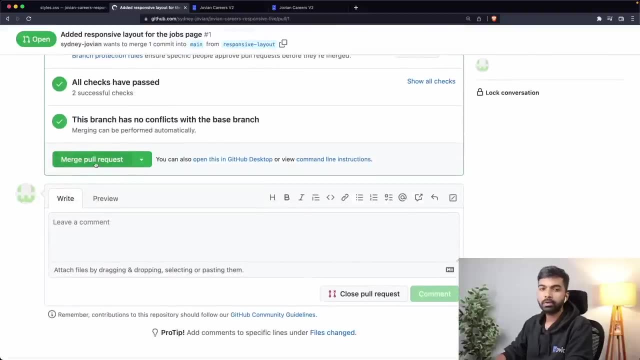 also, this is a good way for you to even do a self review before you merge your changes to master And once the changes are approved, then you can go in and you can get an approval and then you can merge this pull request to master. 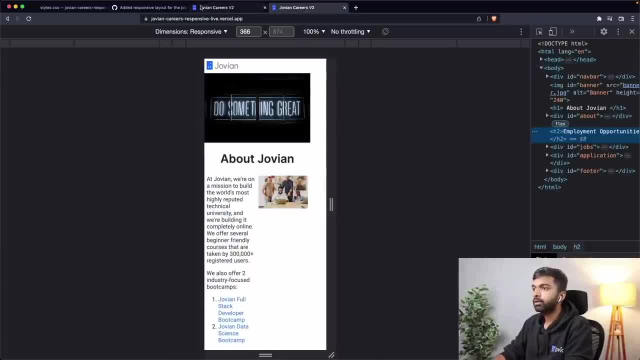 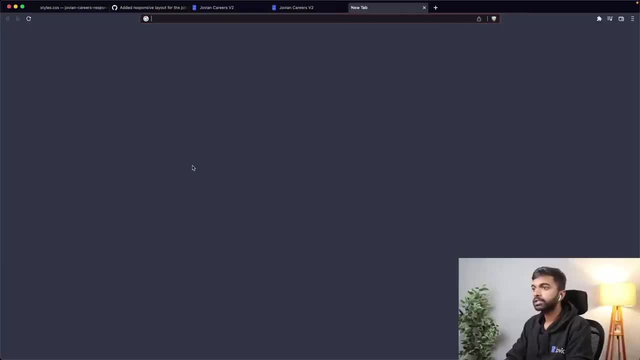 Now, as soon as the pull request is merged to master, what Vercel is going to do is it's going to pick up the new changes from the master branch and it's going to create a new deployment. You can check this on Vercelcom. 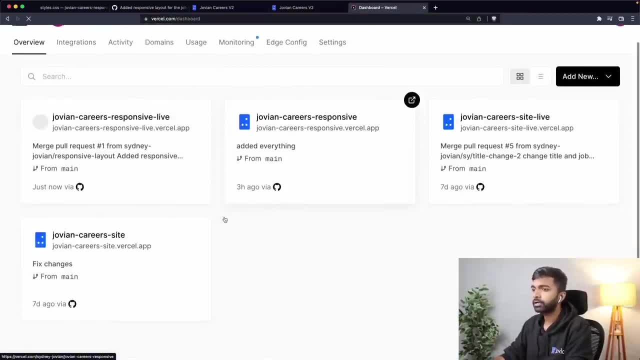 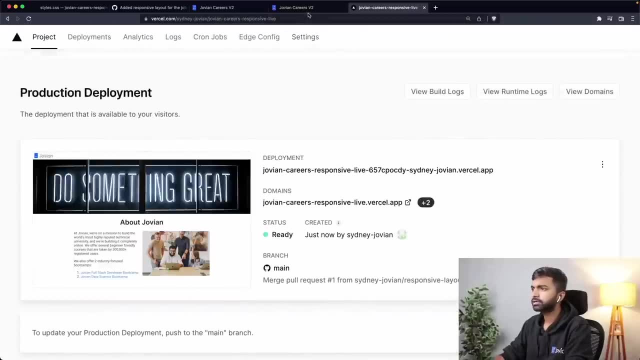 Okay That it is going to create a new deployment Just now. you can see here that's creating a new deployment created just now by Sydney Jovian. And now, if I reload the page, notice that I'm on the deployed main branch- Jovian careers. 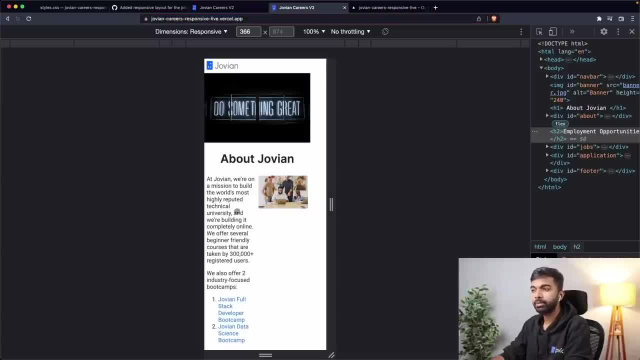 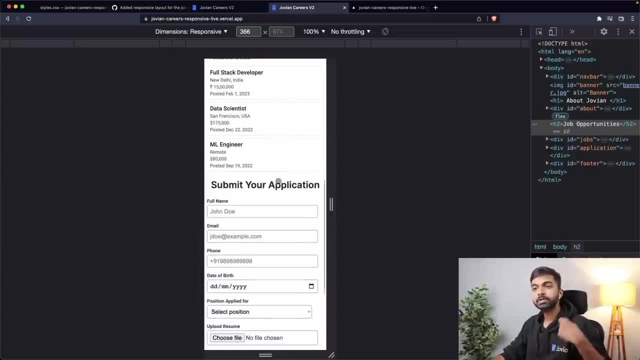 responsive liveapp or Vercelapp and I reload the page and the layout is fixed. This is the layout Now the main page has gone live. So this is the workflow that you need to get used to Create a branch. Do your work. 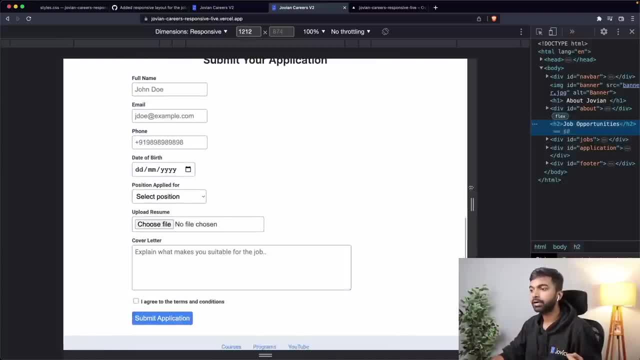 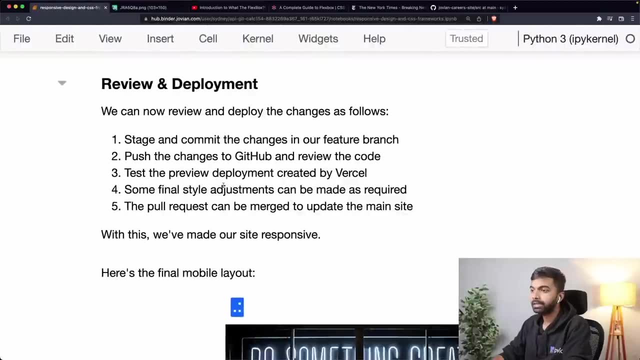 Test it out in a preview deployment and then merge it. then your layout is going to be fixed. Now we've created a responsive design just like that, And that is something that you're going to experiment with in your next assignment. So we staged and committed the changes, pushed the changes to GitHub, reviewed the code tested. 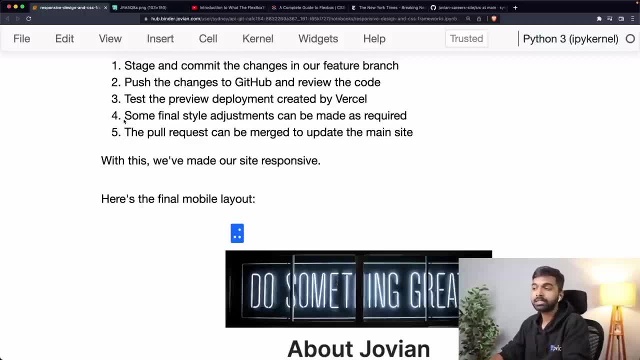 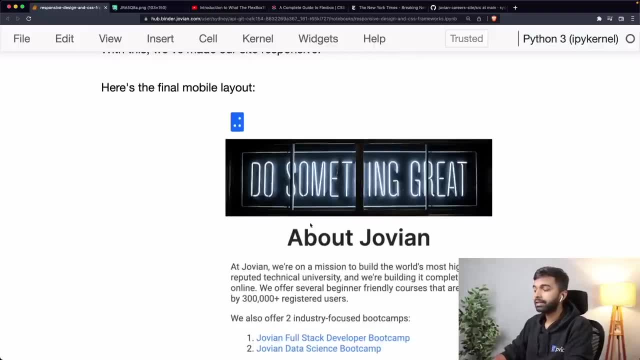 the preview deployment made some. if we can require, we can make some final adjustments, iterate on it, and then the pull request can be merged to the main branch and it gets deployed. And this is the final mobile layout. I think this looks pretty good. 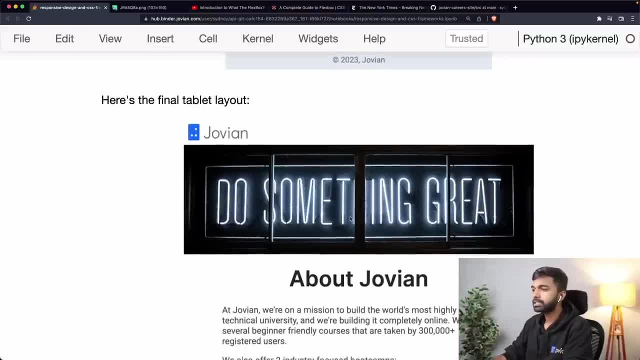 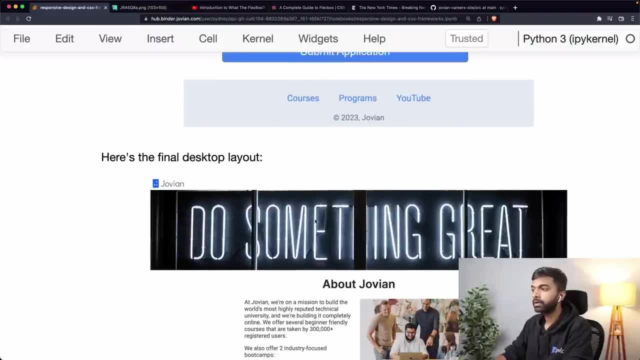 It's: everything is readable, everything takes up sort of the full width. This is the final tablet layout. So we're centering the content on the page to about 500 pixels. we're limiting its width so that things are still readable. And this is the final desktop layout. 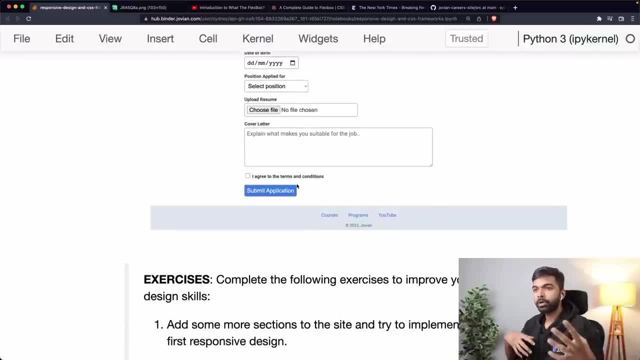 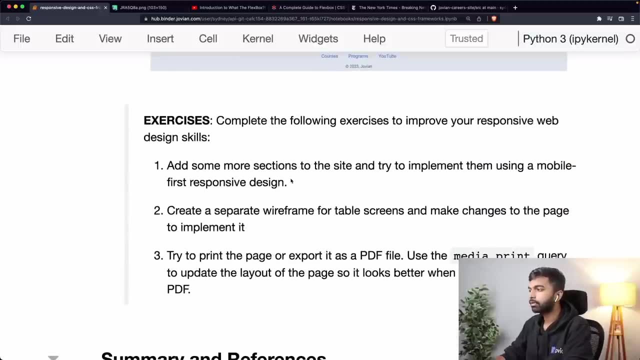 Notice that we did not have wireframes for tablet, but we just use some components from this side and some from that side to build it And, as an exercise, try adding more sections to the site. try to implement them using a mobile first, responsive design. 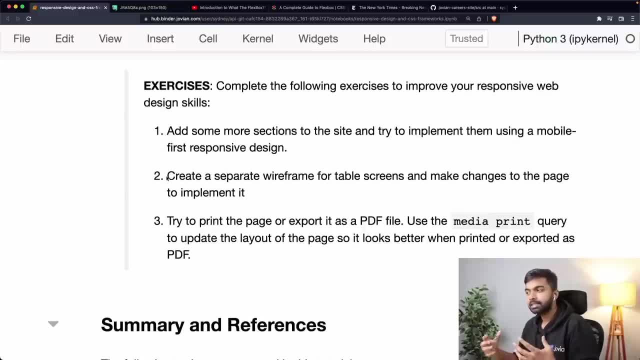 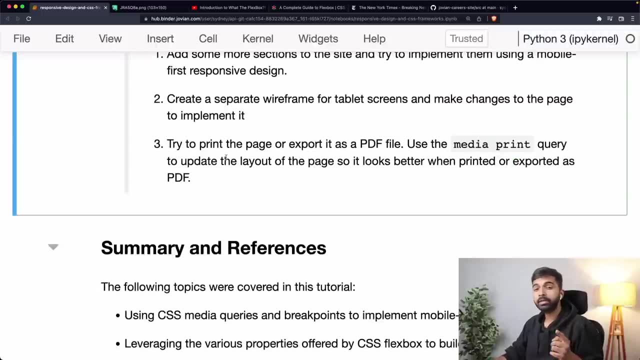 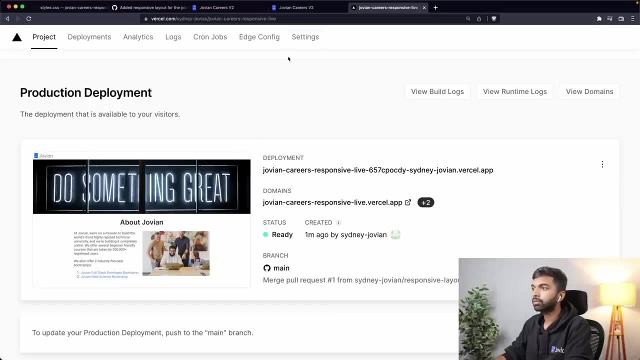 Okay, Okay, Try creating a separate wireframe for the tablet screens and make changes to the page to implement it. And then, one other thing we did not look into was the media type print- what happens when you try to print this page. So you can do that by trying to do command P and then trying to save it as a PDF. you'll. 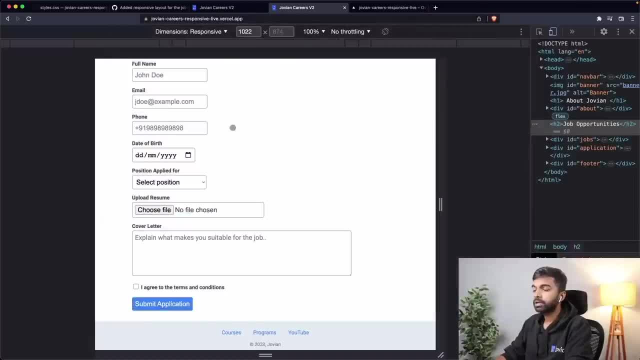 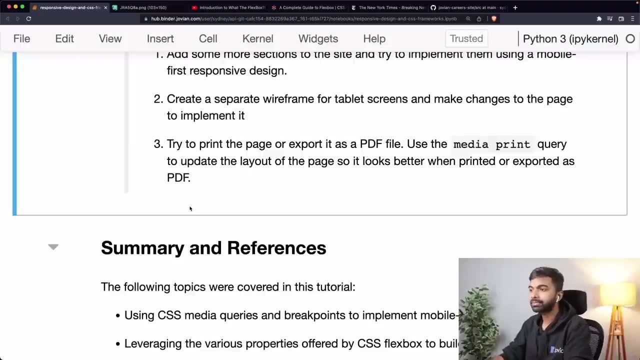 see what your page is going to look like. So by default it just picks up whatever is going to show up on the screen, but for a printout You only need to do a separate layout, And that is something that you can experiment with. that is something that you can experiment. 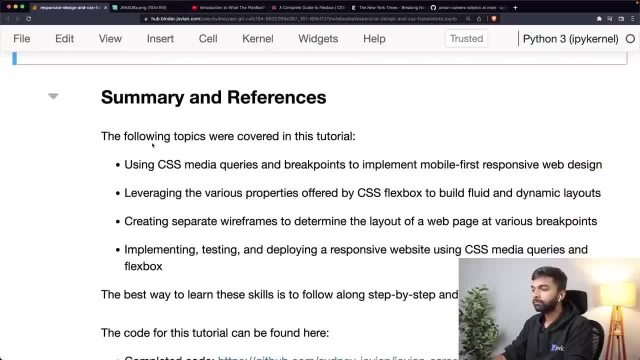 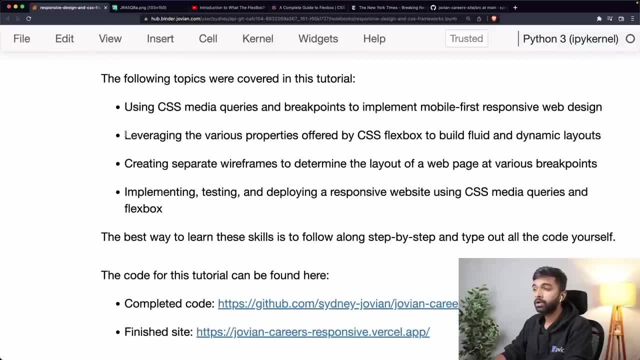 with the media print query. Okay, So that's everything for today. We looked at how to use CSS media queries and breakpoints to implement a mobile first, responsive web design. We looked at how to leverage various CSS properties, specifically Flexbox, to build fluid and dynamic. 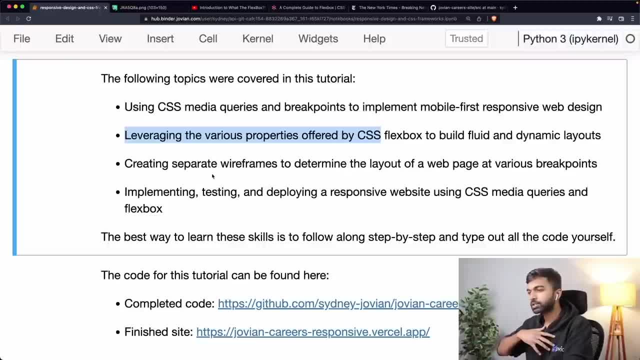 layouts. It's a lot of practice, So we will use Flexbox extensively over the next several months. So don't worry, It's a lot of practice. We looked at how to create separate wireframes or design mockups to determine the layout. 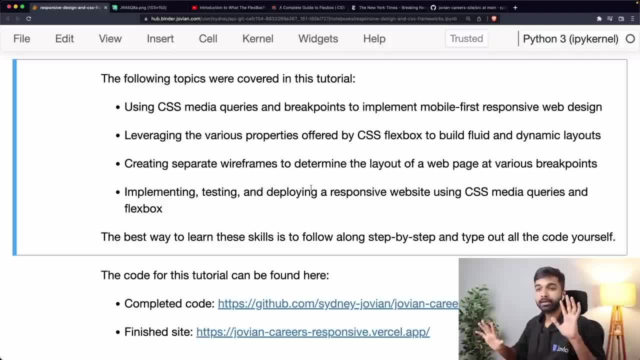 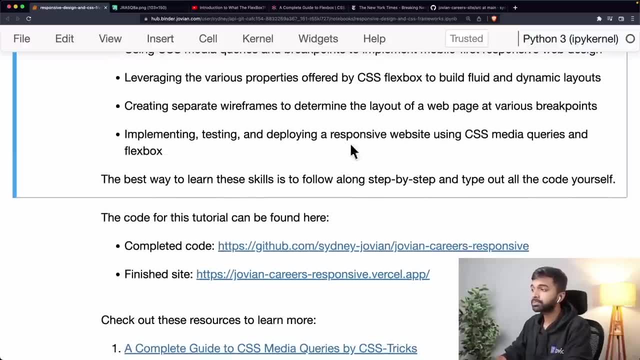 of a web page at various breakpoints. You always, always- should separate the design and the implementation. Don't try to do them both together. You will get stuck. We looked at implementing, testing and deploying a responsive website using CSS, media queries and Flexbox. 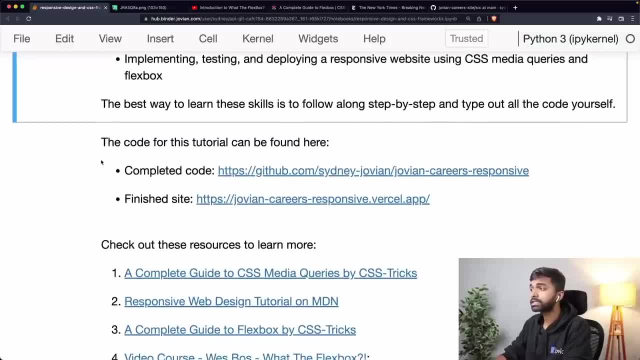 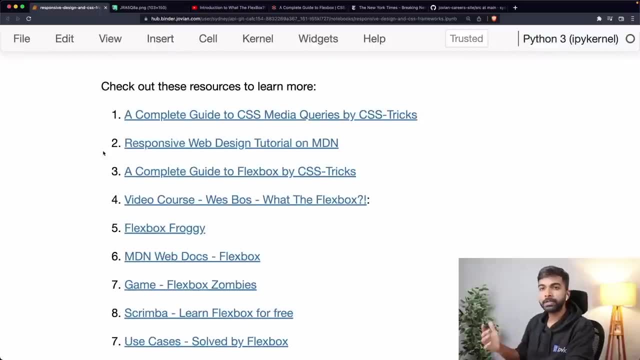 And the best way to learn these skills is to follow along step by step and type out all the code yourself, And you can check out the completed code here using these links. I have included a ton of resources here. The idea is that you can do it yourself. 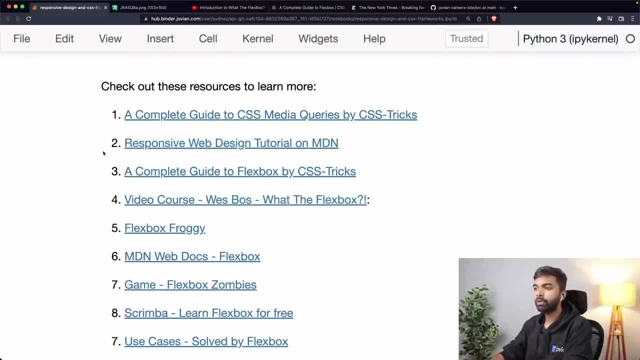 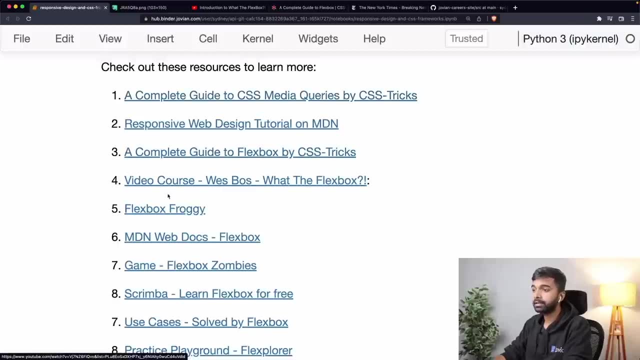 The idea is not that you need to go through all of these resources right now. A few I would recommend, though, is a responsive web design or media queries tutorial on CSS tricks, The video course by Wes Boss on what the Flexbox, But there are a bunch of others. no matter what you are feeling under, feeling scared- 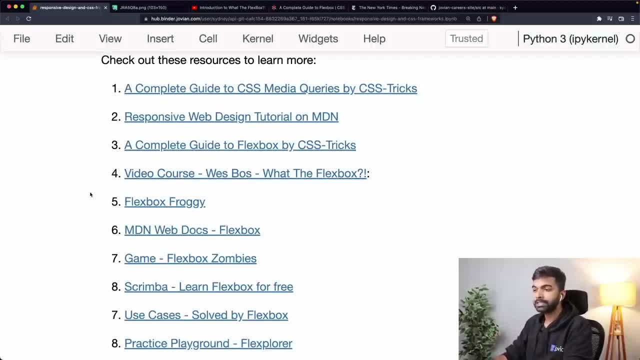 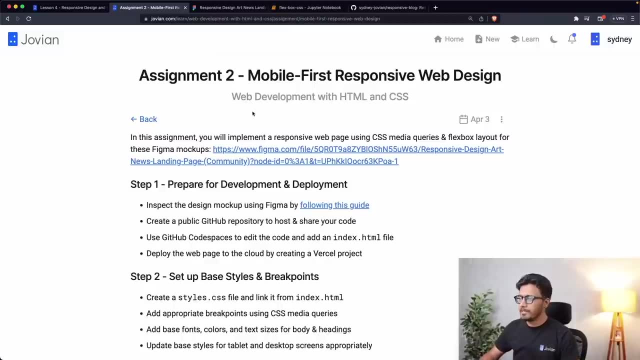 about, or not confident about or doubtful about, check out one of these resources, You should be able to figure it out. if one of the concepts that we covered today did not make sense, And that's it. In this assignment 2,, you will be implementing a responsive web design using CSS media queries. 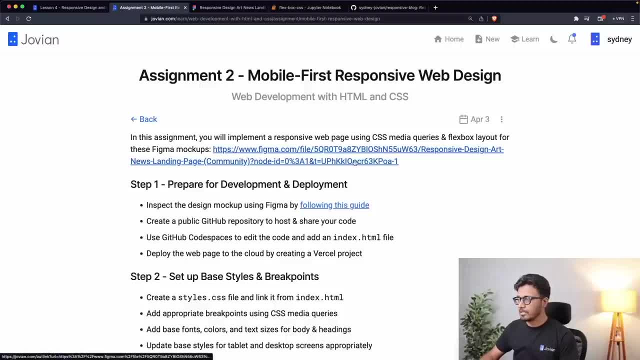 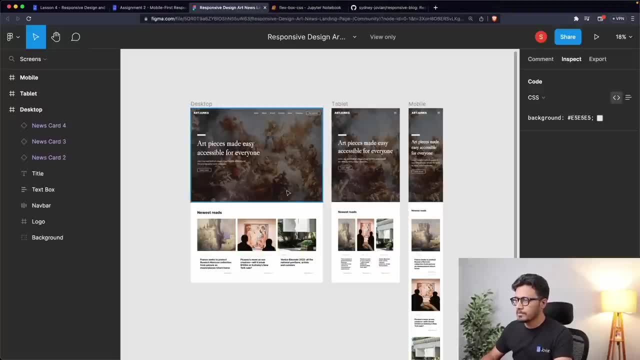 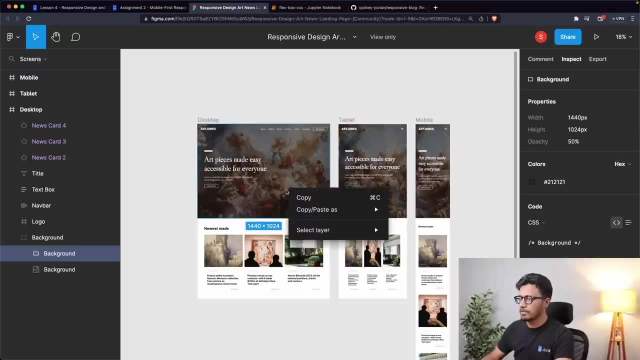 and Flexbox. So the Figma mockups are already provided to you. Let's quickly go through the mockups. So in these mockups there are three layouts: for desktop, tablet and mobile, And on the desktop view there is a navbar. 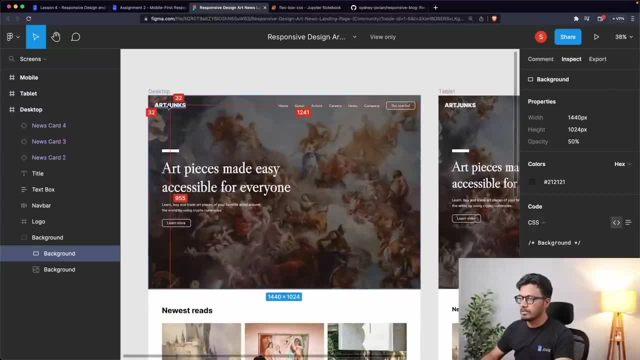 With the text you can see the layout And on the desktop view there is a navbar. And on the desktop view there is a navbar With the logo of the company and some graphics, some title, subtitle and learn more button. 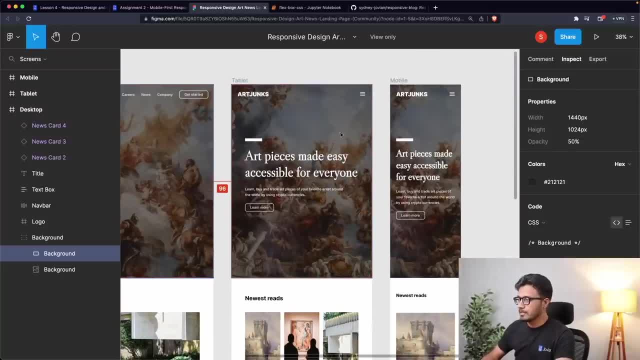 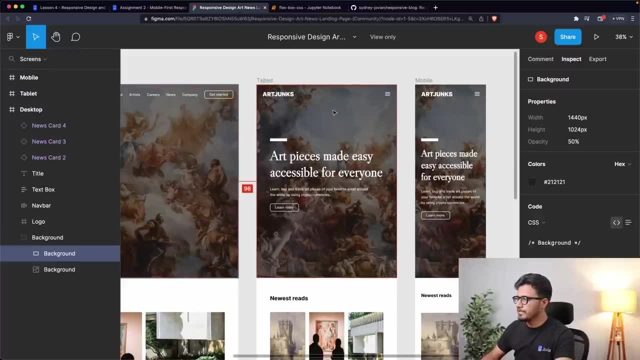 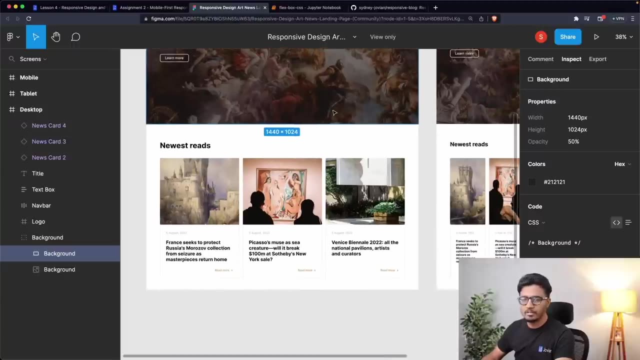 And on the tablet and mobile view also, there is similar layout, but the navbar is different. It is not completely visible, It is in the collapse mode And below the hero section we have the newest read section, Which is a card layout. 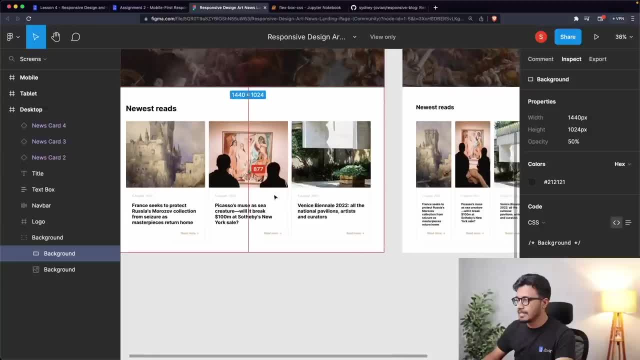 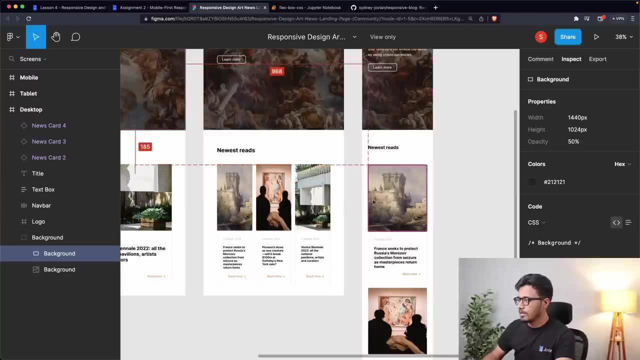 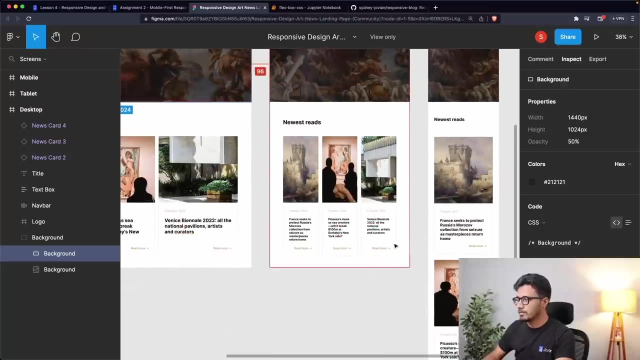 And on the desktop there are three cards in a row, And similarly on the tablet also there are three cards in a row, But on mobile we can see that the layout is a bit different, So it is having a column layout. 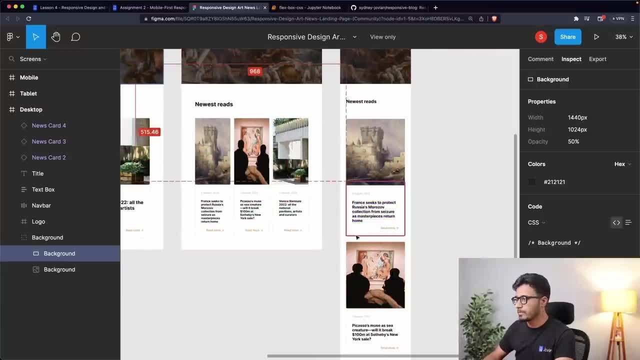 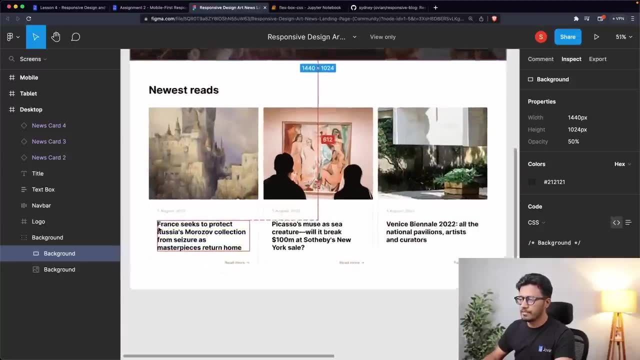 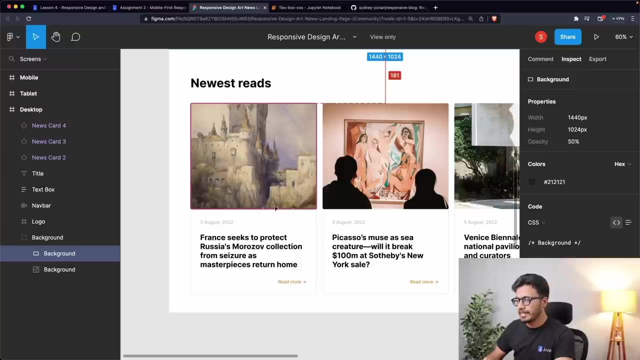 So you will need to use some flex properties maybe to design these layouts for different devices. And inside the card, if we zoom in, we have few more elements: The image for the article, the date of publish and the title, and read more link. 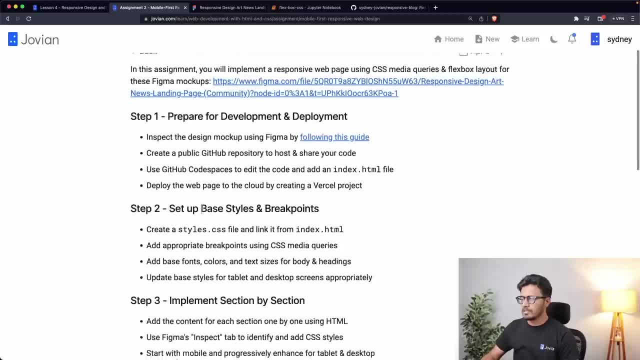 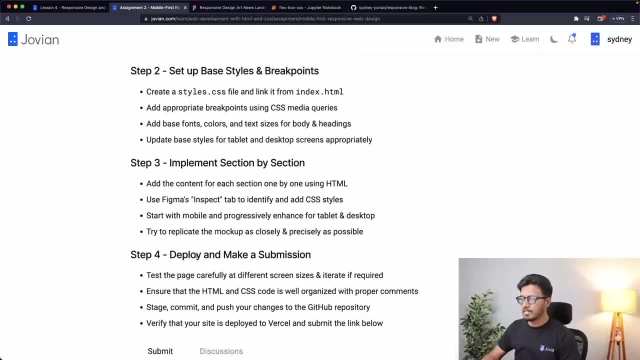 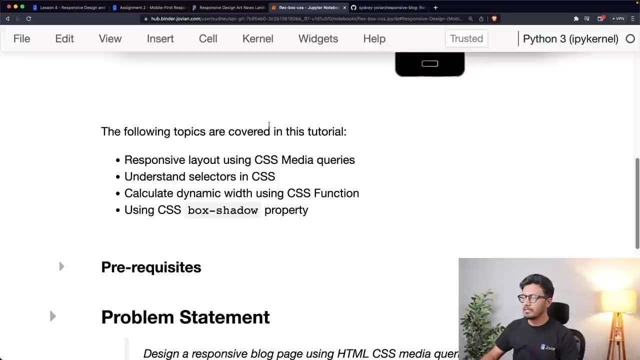 So this is how the assignment tool is looking. The steps to proceed with this assignment are already mentioned And I hope you guys have already started on that. So, coming to today's session, Today we are going to build a responsive web page using flexbox and media queries. 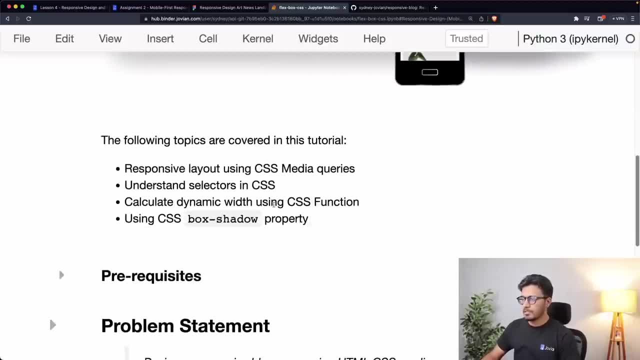 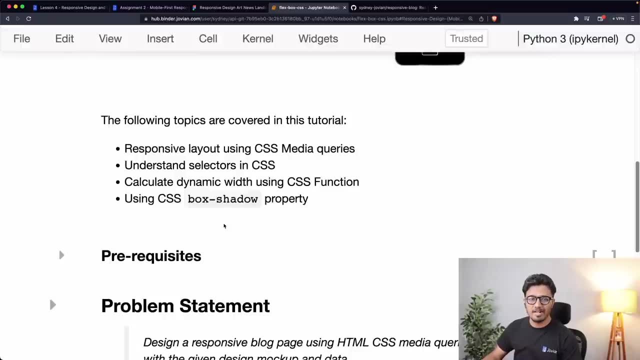 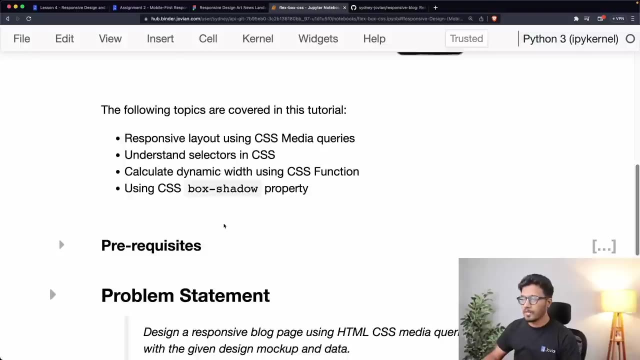 The following topics will be covered in today's tutorial. So we will be designing a responsive layout using CSS media queries. then we will understand what are selectors in CSS and how to calculate dynamic width for particular elements using CSS functions. And in the next video we will discuss how to make a responsive layout using the box. 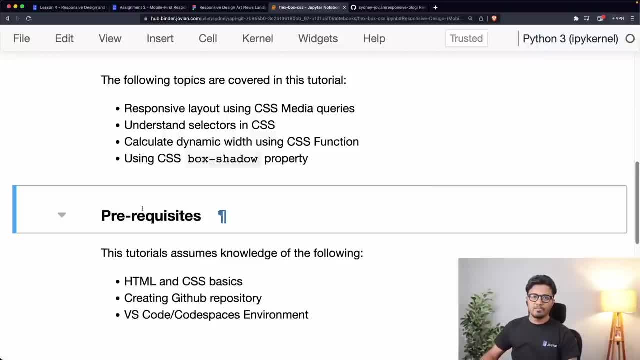 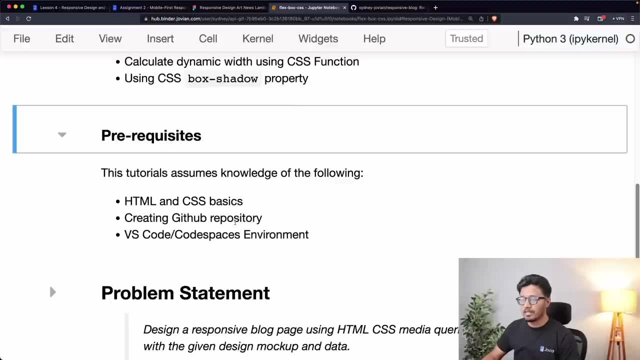 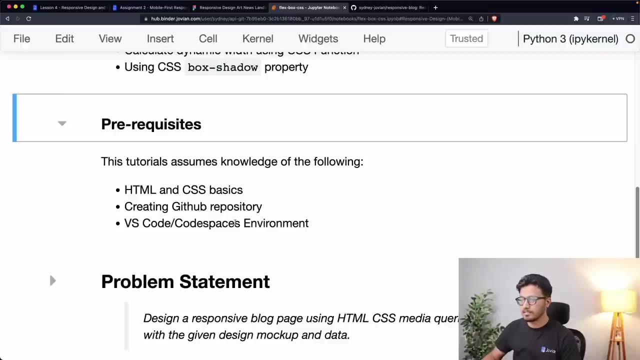 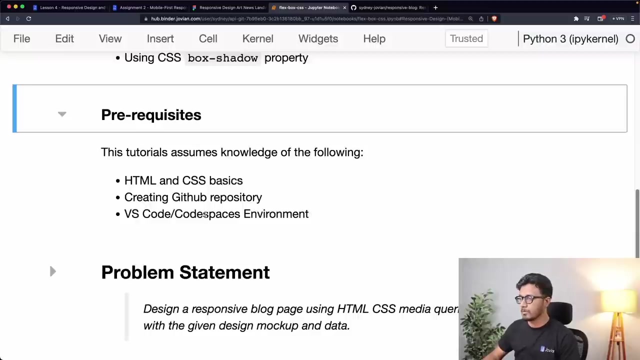 shadow property. So the prerequisites for today's session are: you should be aware about basic HTML and CSS And you should know how to create a GitHub repository, And the environment that we are going to use for today's session is VS code, And we will be using the cloud base VS code, that is, the code spaces which is provided. by GitHub. So, as a point of view, we are going to use the code spaces. So in the next video we will be talking about how to build a GitHub repository and how to use it and how to create a GitHub repository. So, as a point of view, we are going to talk about how to build a GitHub repository and how to create a GitHub registry and how to create a GitHub repository in a single comment. 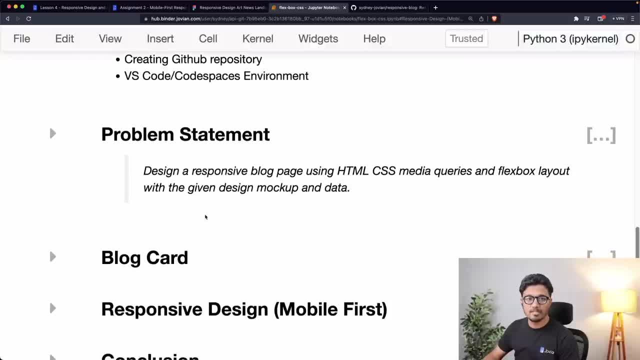 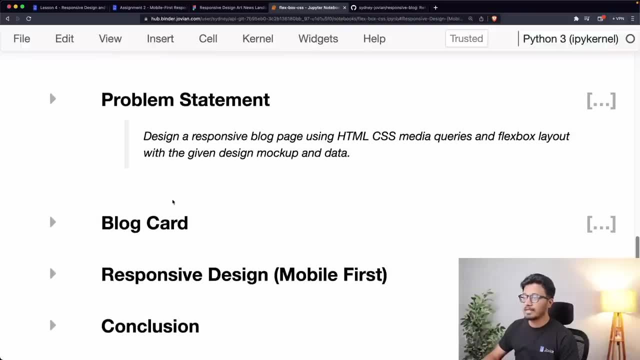 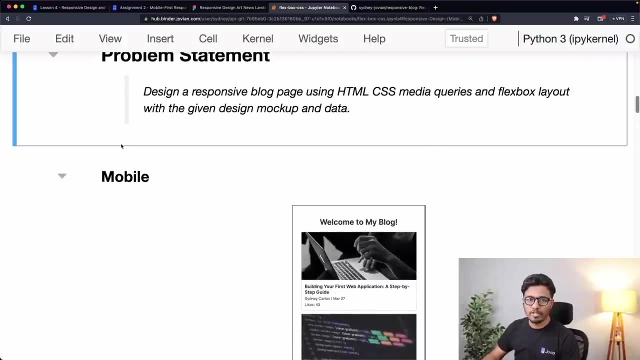 part of designing a web page. we are going to design a responsive blog page which will make use of media queries, flexbox layout, and the design mockup and data is provided for you. so let's go through the mockup quickly. so this is how the layout will look on mobile. 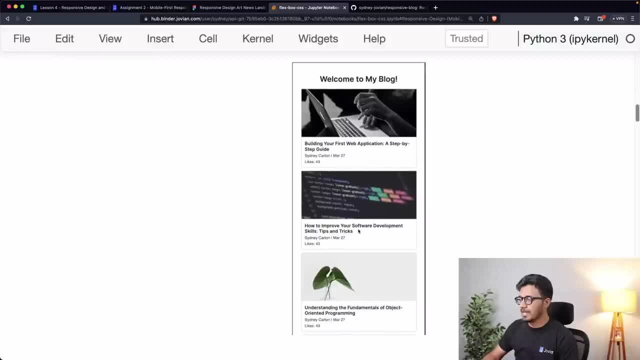 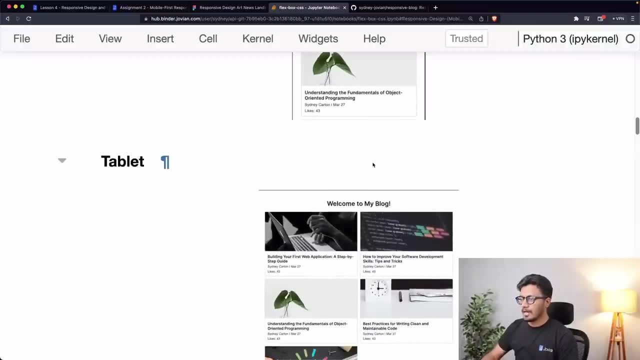 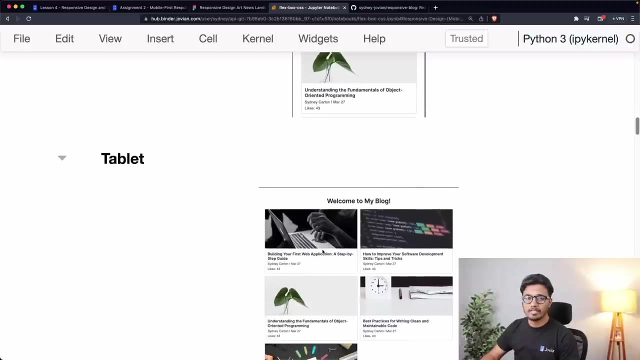 it will have a page title and it has the cards which are stacked vertically. so this is basically a column layout. you can see, and on tablet we can see that the card layout is almost similar, but the method of rendering is different. so we can see that on the tablet there are 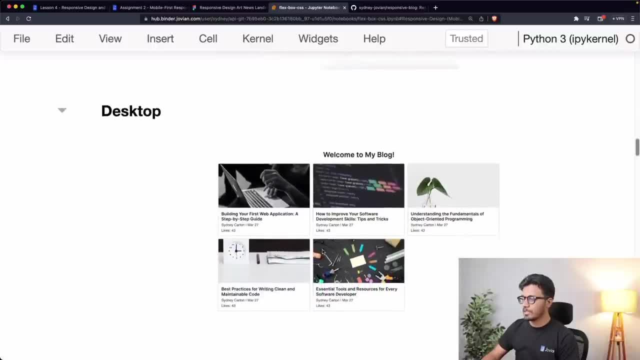 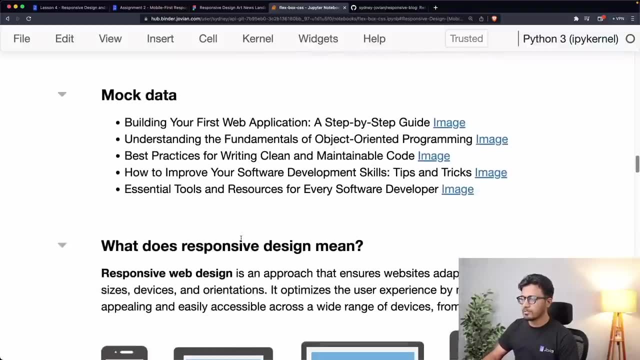 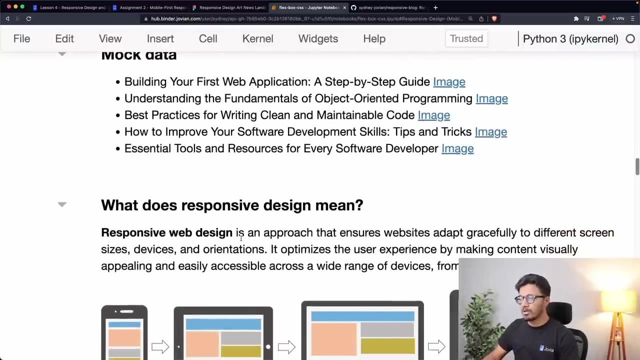 two cards in a row and for desktop it will be three cards in a row. so this is the layout. this is the mock data that we will be using for our today's session. so first let's quickly recap about what is responsive design. so responsive design is an approach which ensures that our 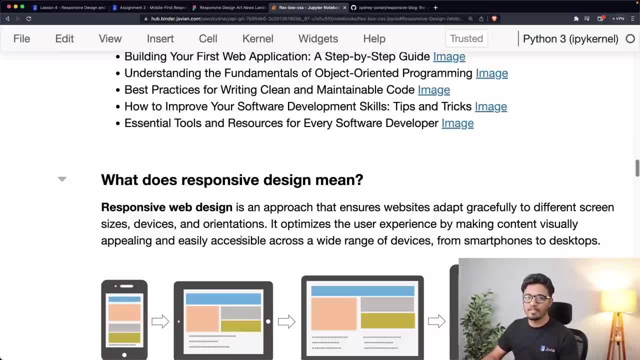 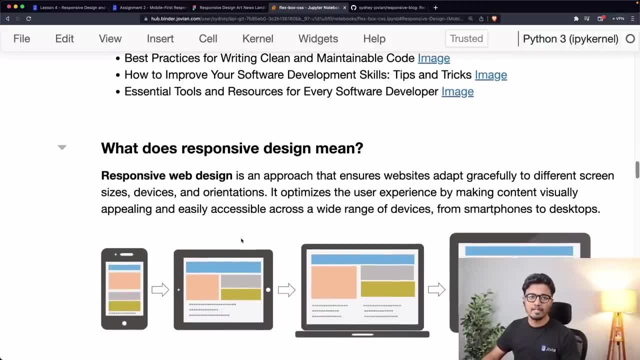 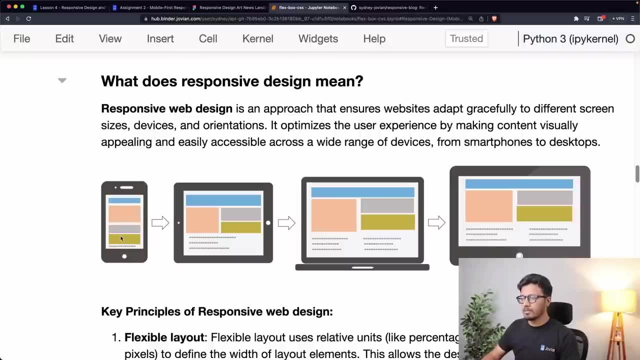 websites will look correctly and adapt to various different screen sizes, devices and orientation, so it will optimize the user experience by making the content more visually appealing. so you can see from this image that this is some example of the mockup. so on mobile it is vertically aligned and when it when we change the device, it automatically gets aligned to some different. 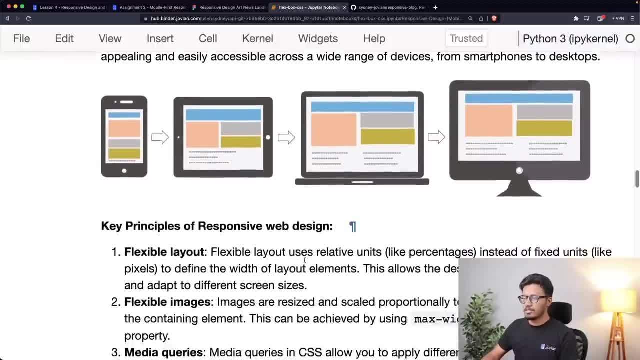 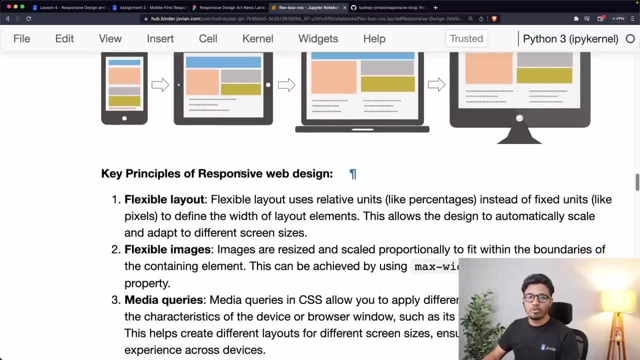 layouts and it gets scaled on higher devices. so there are few key principles that we should be aware about responsive web design. first is the website layout should be flexible. it should not be fixed. sized like the width should not be given in pixels if we resize the screen. it should. 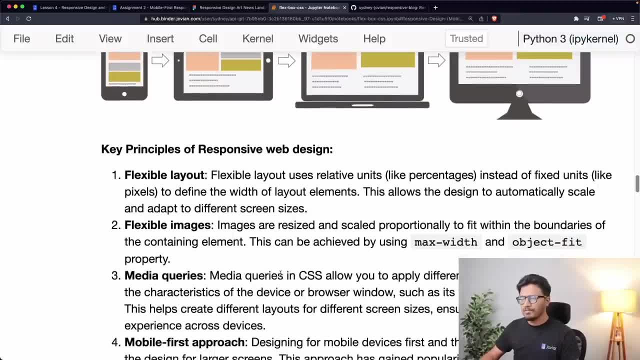 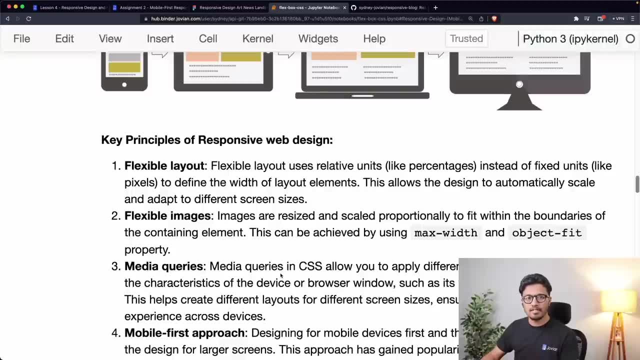 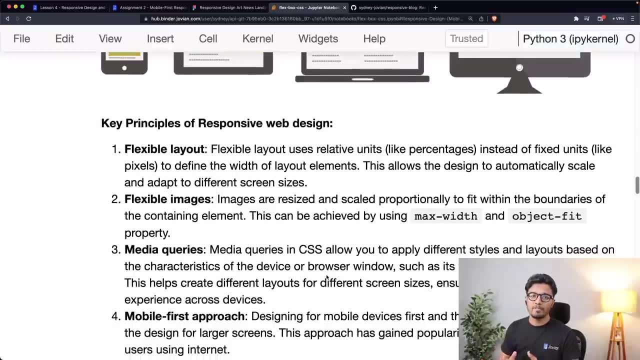 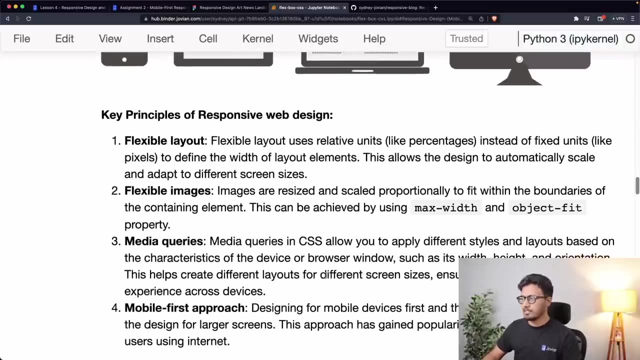 get scaled accordingly. next is the flexible images. so images have their own size and when we import the external images, they render directly. if we don't specify the width and the height separately and it might happen that the image can overflow. uh of the screen width. ensure that this doesn't happen, we should be using some css properties. so one is the max width that. 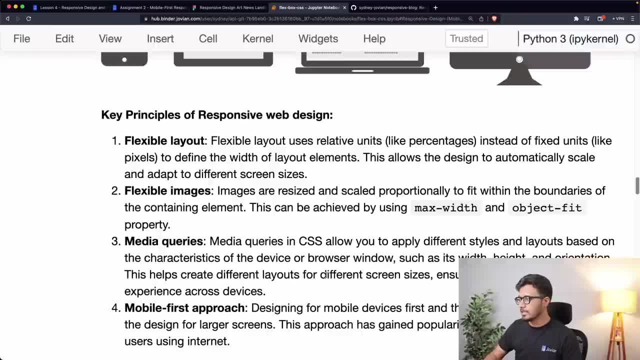 will ensure that our image is within the screen width and other is the object fit that you might have already used in the previous lectures. so that is used to maintain the aspect ratio of the image and it makes ensure that the image doesn't get stretched. so we will be using that today. 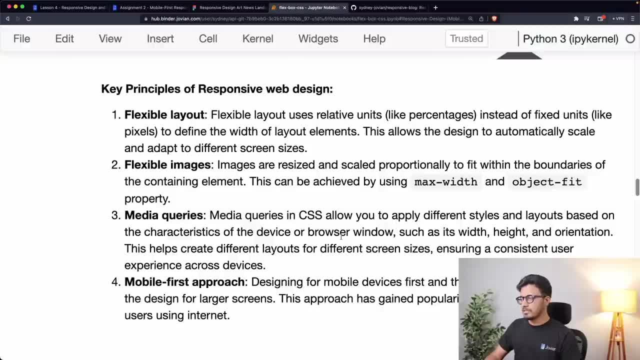 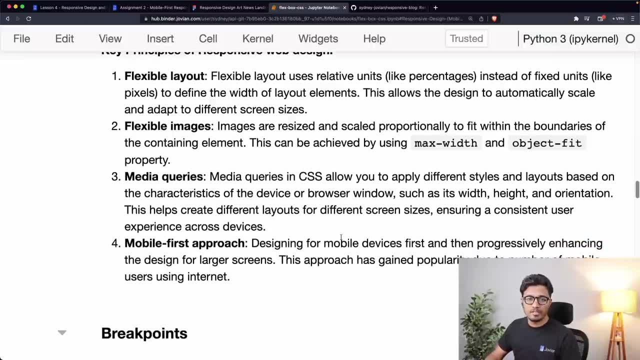 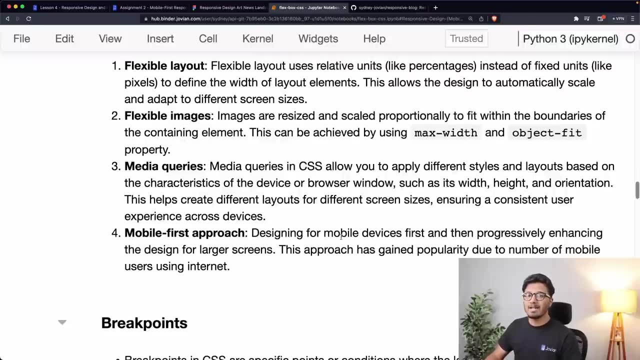 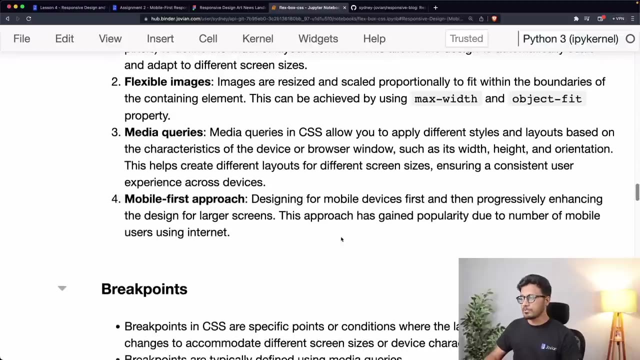 the third thing is the media queries, which allows us to write various styles based on the layout of the device, so we can specify various device properties like width, height and orientation and write the styles for that particular query. fourth is the mobile first approach. so this approach tells us that we should start designing our 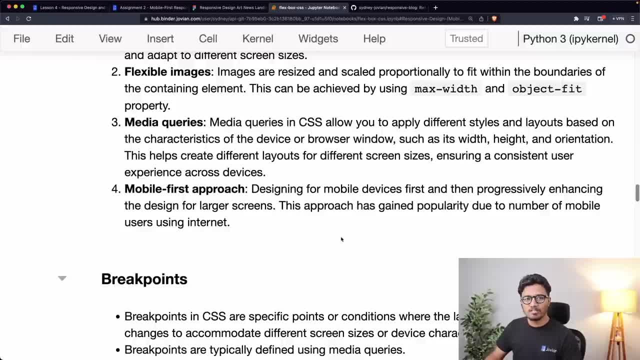 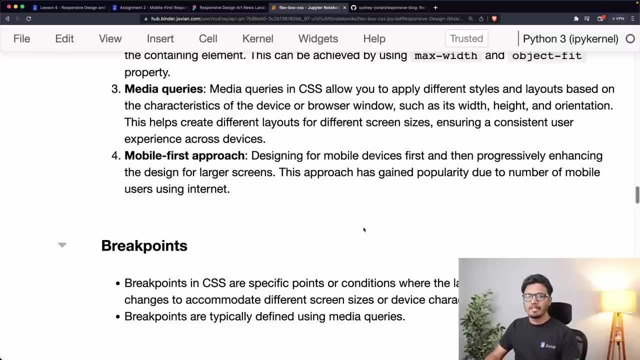 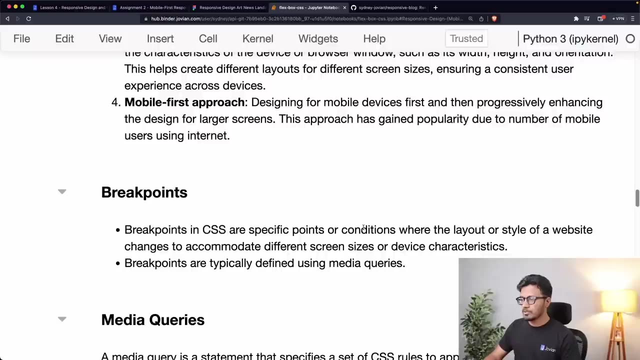 web page from mobile devices and then progressively enhance to the larger devices like tablet and desktop. so this approach has gained popularity because of the number of users of mobile devices compared to other devices. so the next concept is the breakpoints. that is also important in responsive web design. so breakpoints in css are specific points or conditions. 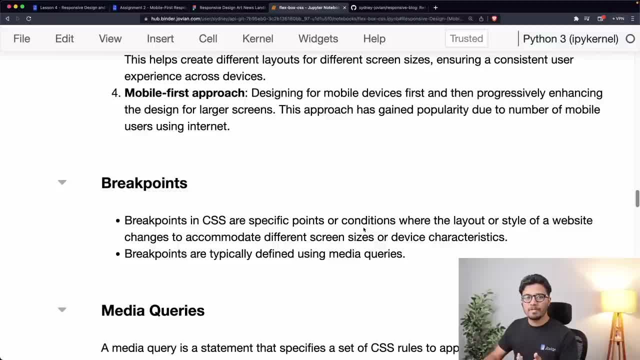 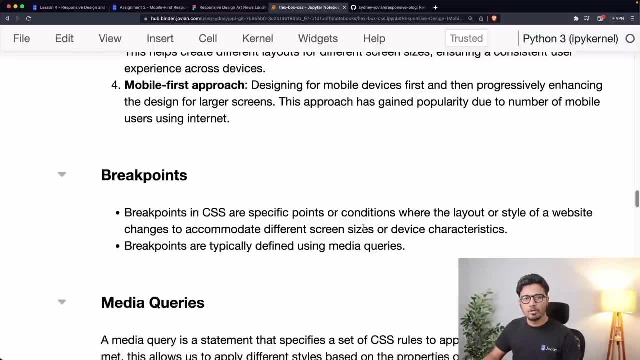 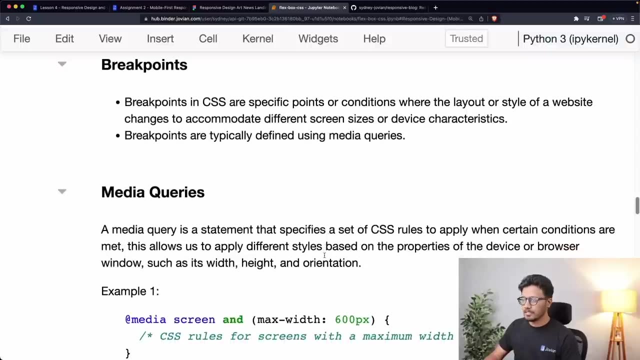 where the layout or styles of our web page are going to change and accommodate to different screen size. these breakpoints are generally used along with the media queries. so what is media query exactly? so media query is the statement that allows us to write a specific set of css rules. 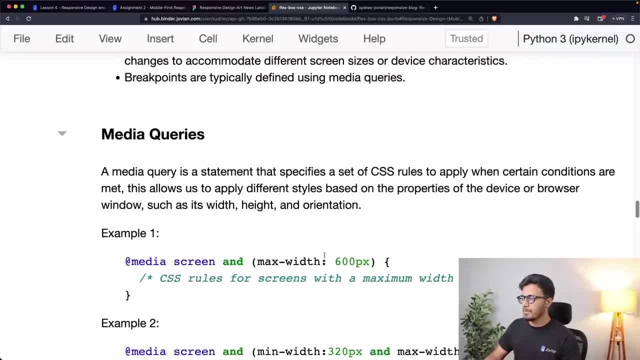 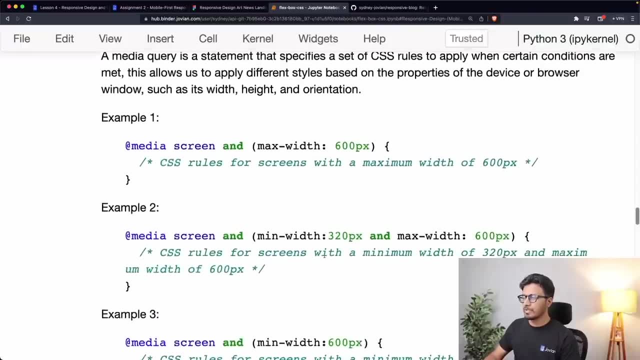 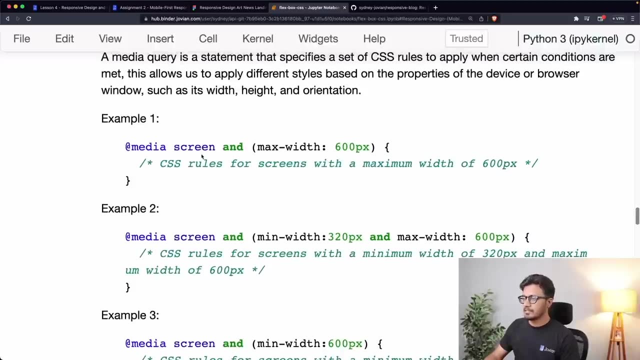 when certain conditions are met. so these conditions are based on the width, height and orientation of the device. so let's see few examples quickly. so in this example one we have a media query which says that it should apply to the max width of 600 px. so whatever styles we will write inside this block will apply to all the devices whose width 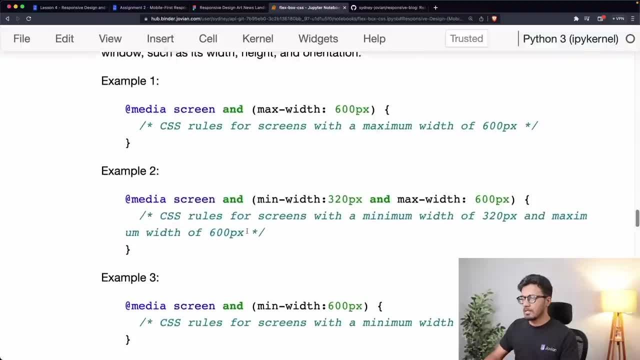 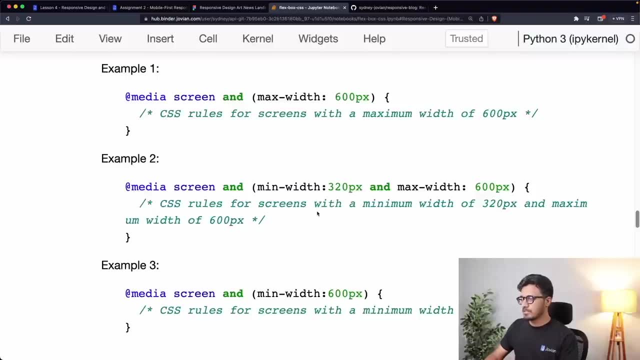 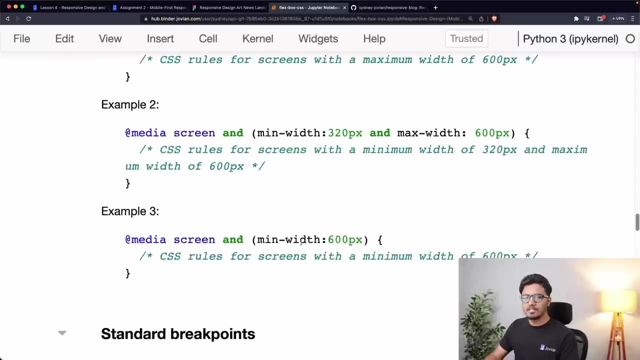 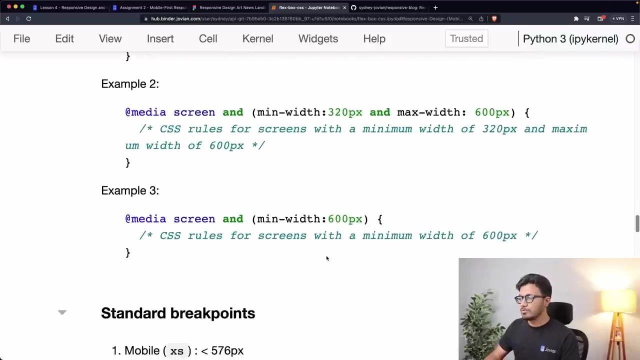 is less than or equal to 600 px, and this example tells us that we can also specify min width and max width together, so these styles will apply for all the devices whose width is between 320 px to 600 px. and third is the min width, which will apply all the styles for the devices which whose width is 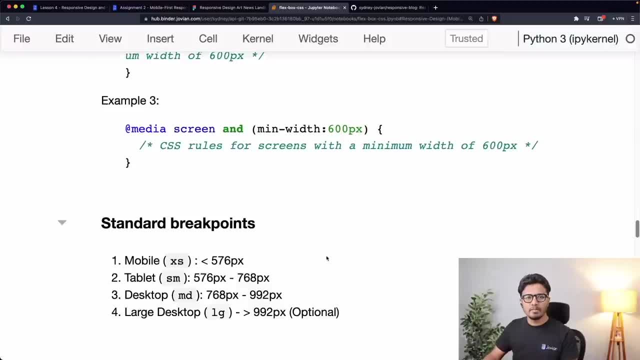 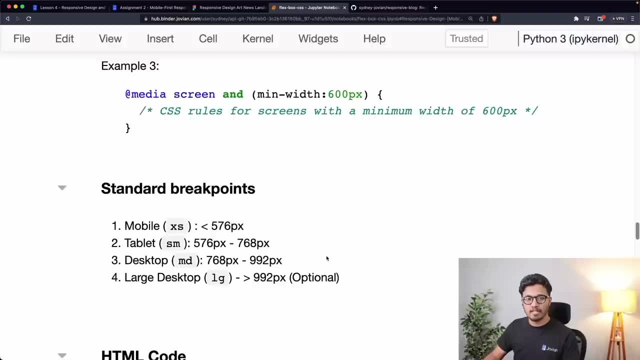 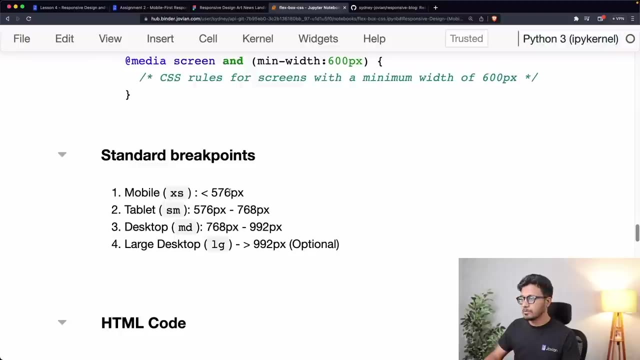 greater than or equal to 600 px, so we can use any arbitrary width and height for defining these media queries, but there but there are few standard breakpoints that are generally followed based on the device type types. So, for mobile, the width of the device should be less than 576px, and tablet, which 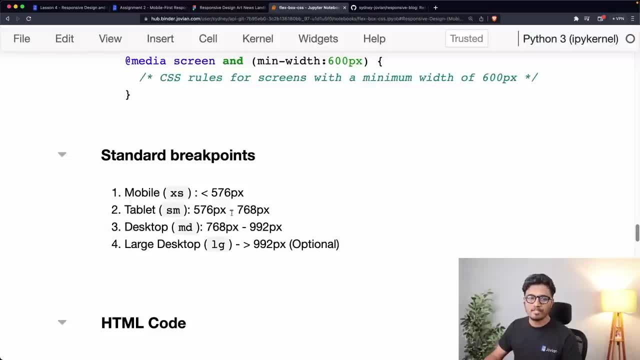 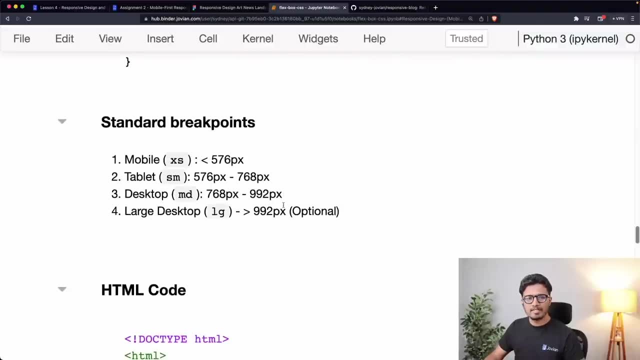 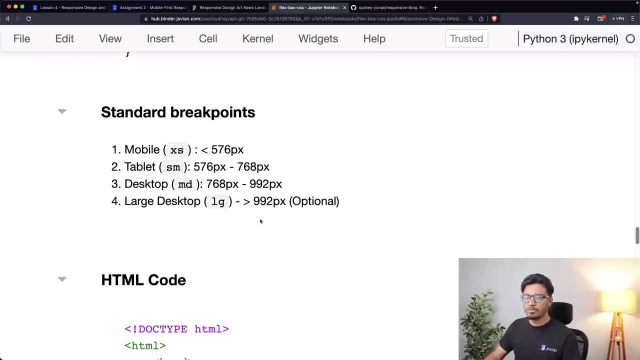 is the SM device. it ranges from 576px to 768px and desktop ranges from 768 to 992, and there are also higher resolution devices, which we call large desktop, whose sizes are greater than 992px. So let's get started with the coding part. So we will be using GitHub code. 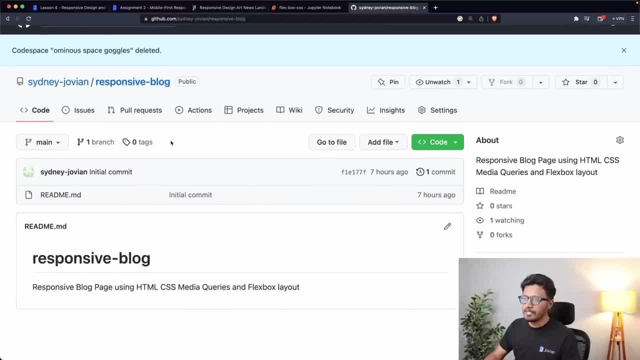 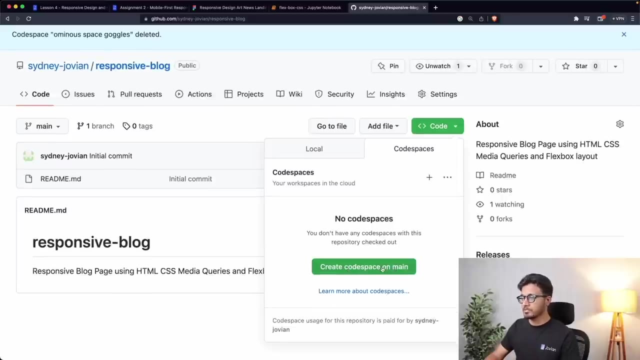 spaces. So we will be needing one GitHub repository- So I have already created a repository here- and to run in the code spaces you just have to click on code and click create code space on main, which the main is the branch of our repository Once you click that. 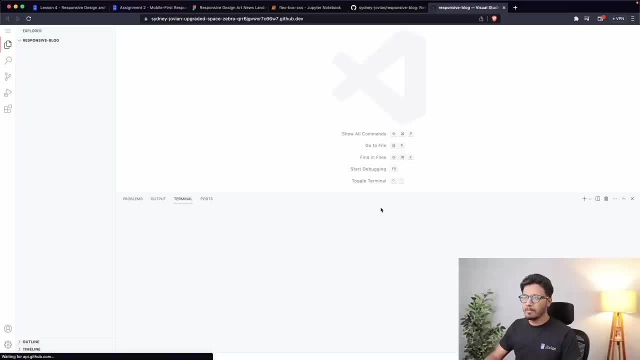 it will open a new tab and you will get a VS Code cloud interface and it should load in couple of seconds. Yeah, so it is loaded, and on the left side you will see the list of files. So we are having a readme file here and we are not going to use the terminal, so 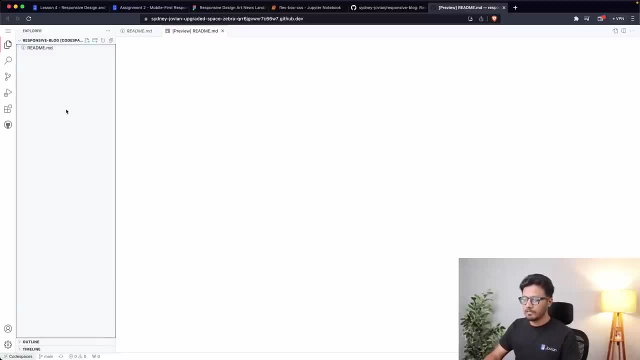 we will just leave it as is and let us quickly write our first file, which is indexhtml. So we will add some basic html code that is required for every html document we write. So we declare the doc type, then the HTML tag. inside this html tag we will be having a head. 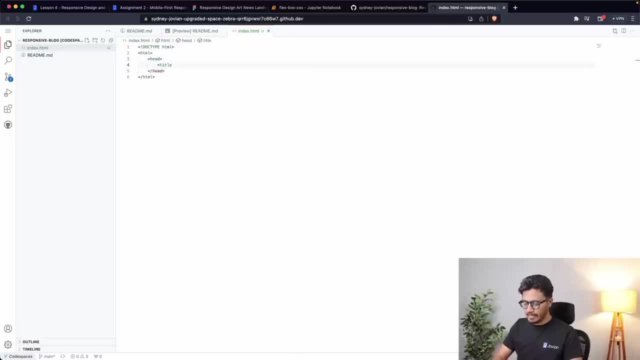 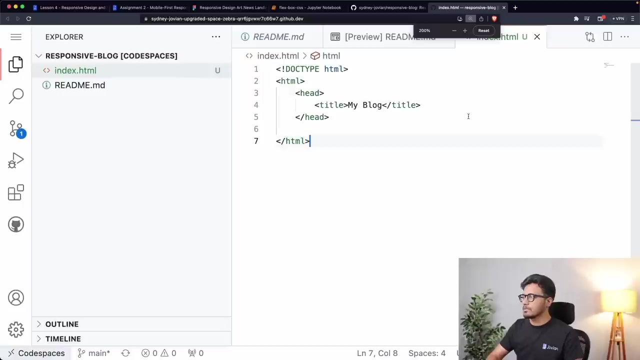 tag tag. we require a title tag, And let me give the title: my blog. Hey, Ashish, can you zoom in a bit? Yeah, A little more. Yes, Okay, Yeah. so, apart from head tag, we also need a body tag, And let me. 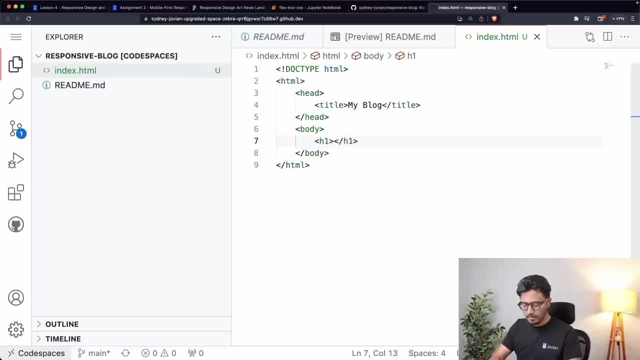 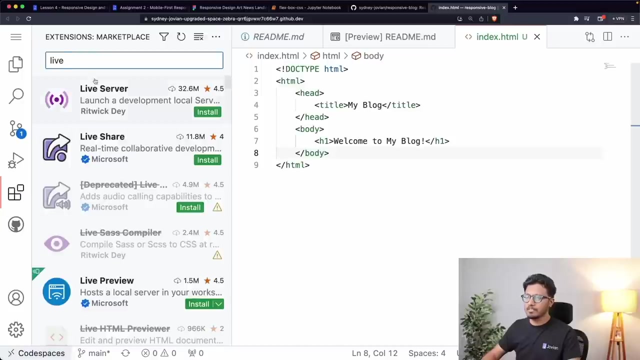 add a h1 tag here, which will be the page title, And alright. so we have written the basic HTML file And to run this file we will need some extension. that is live server, and it can be found in the extensions tab. So there is the. 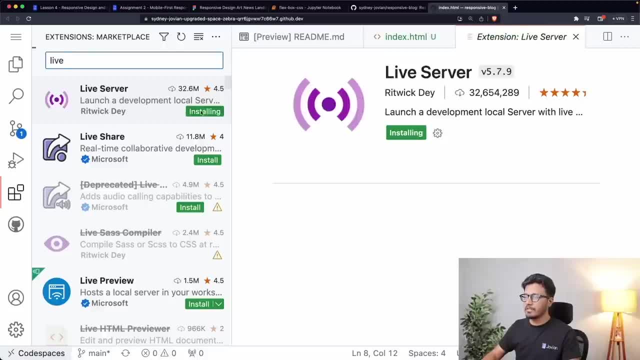 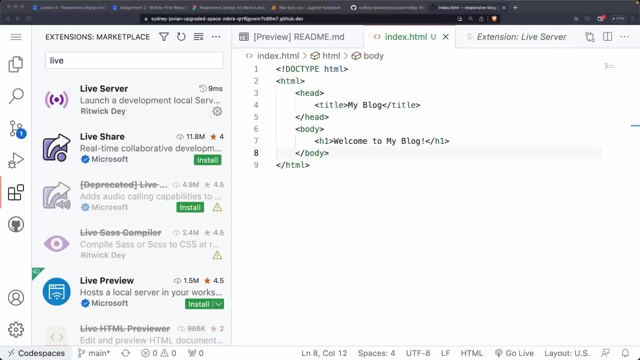 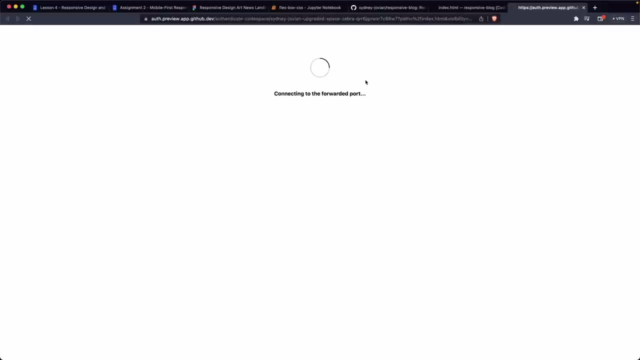 extension live server by big day. we can install that. Yeah, once it is installed, you will see this go live option. Yeah, so you will see the go live option At the right bottom. you can click on this And it will start a server. and it will. it should open in the new. 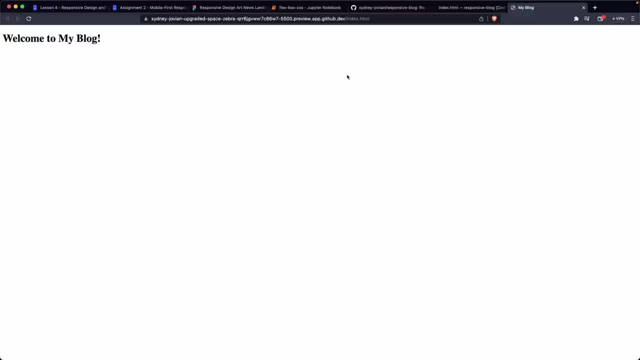 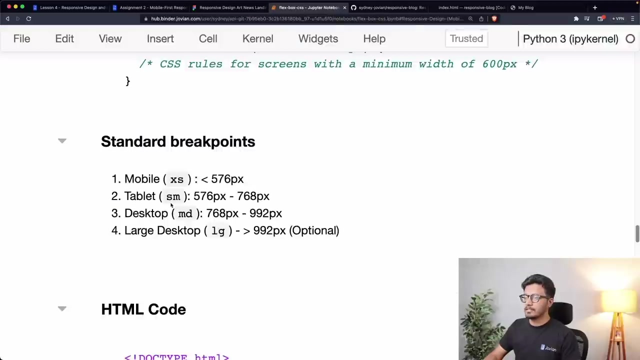 tab, The HTML page that we just wrote So we are able to see. Welcome to my blog. Now let's add some CSS styles. So we will be using external CSS file And we will create one file which is base dot CSS. 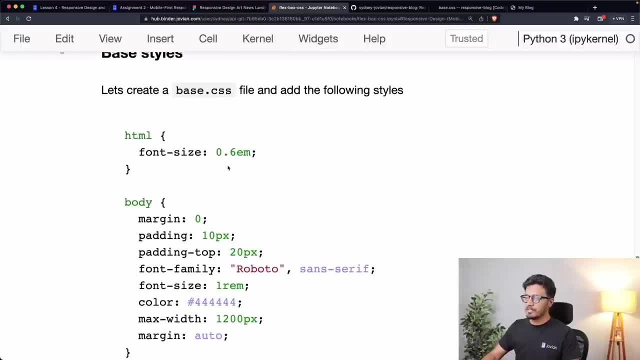 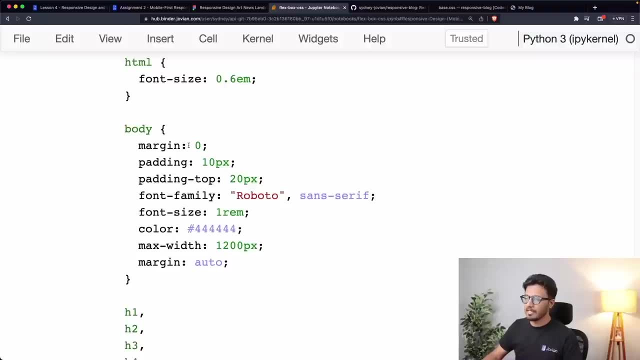 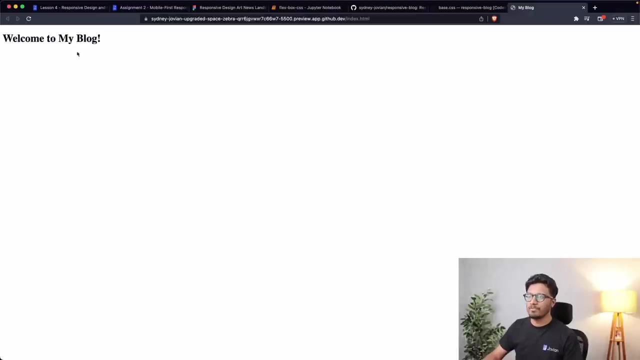 So this base dot CSS will contain all the code that is required to be applied to all the basic HTML tags. So this is important to be consistent across various browsers, because various browsers have their inbuilt style that is auto applied to all the tags. For example, on this blog page we haven't specified any 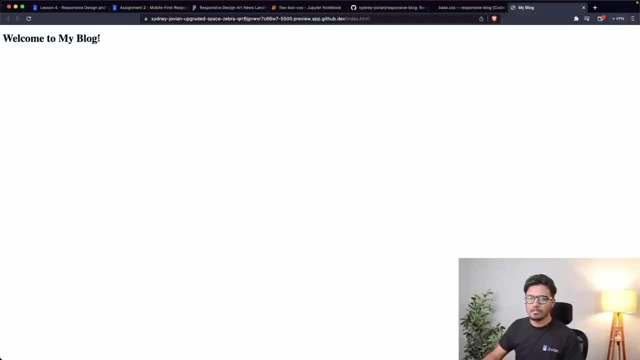 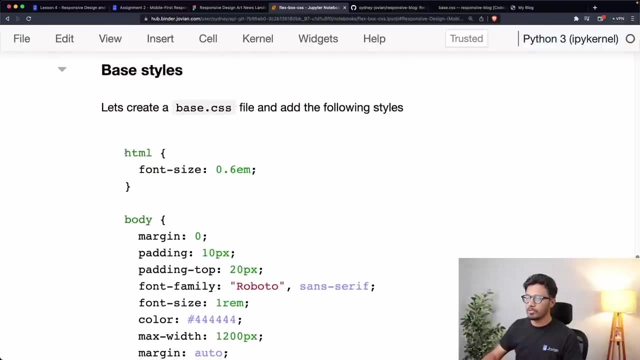 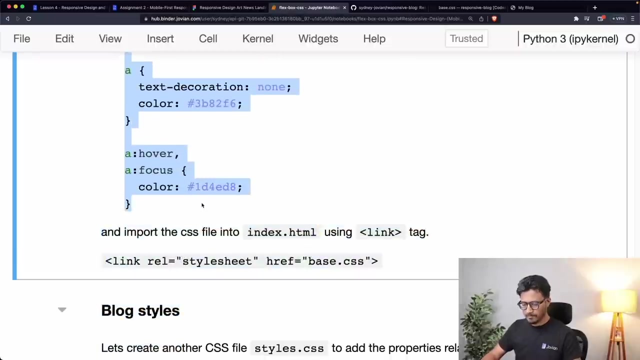 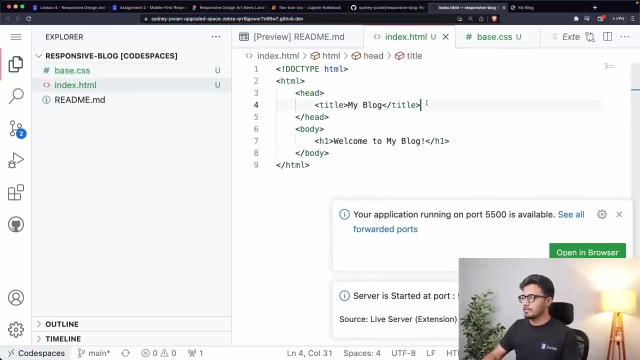 font or any font size, So it is automatically given by the browser. So I will just copy these styles from the notebook And put it into this base dot CSS file And we can import this file using link tag. The site should be style sheet And href should be based on CSS. 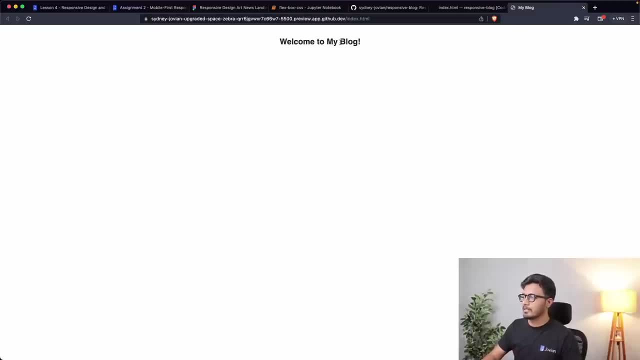 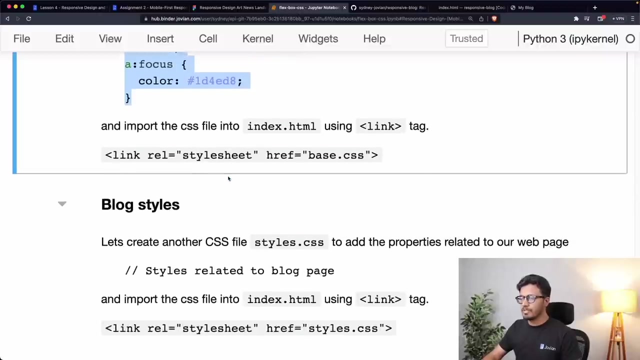 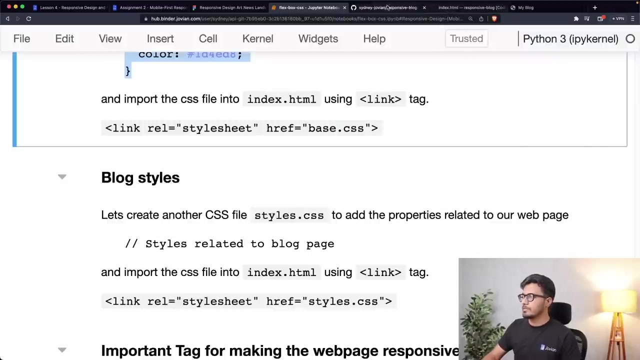 Yeah, So the file is loaded correctly And we can see that the font is now changed to Sans serif And also the title is centered to the page. now the next thing we will do, we will create one more file, which we will call styles dot CSS. so in this base dot CSS file, you can see that there is no code. 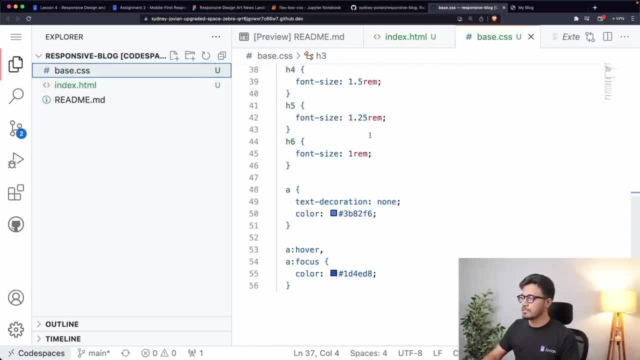 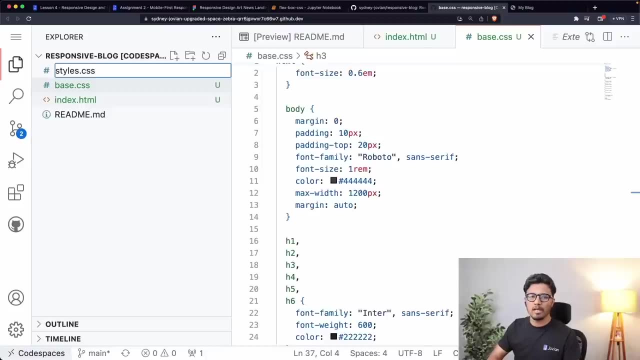 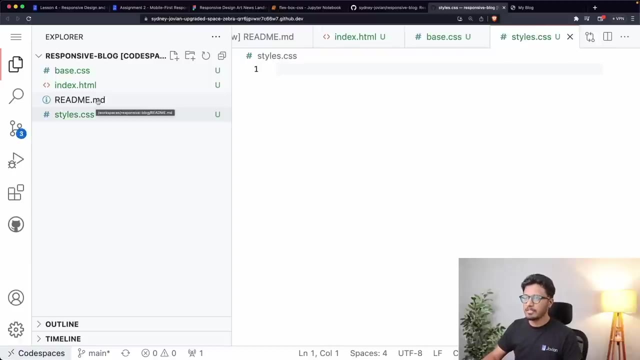 related to our blog page design. so we will create one more file- files, dot, CSS- to write all the application specific code. it's not a mandatory thing, but to keep things more organized and to keep our styles more organized, we can create one more file and it can be similarly imported the way we have imported the. 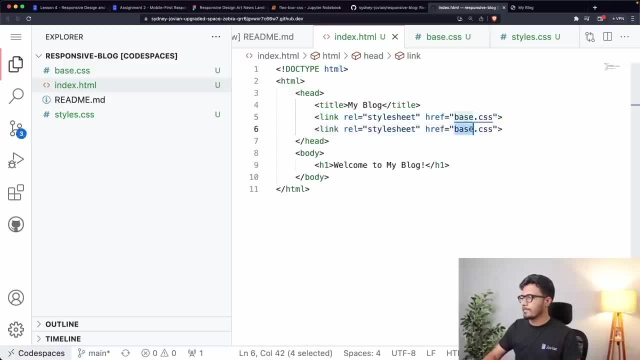 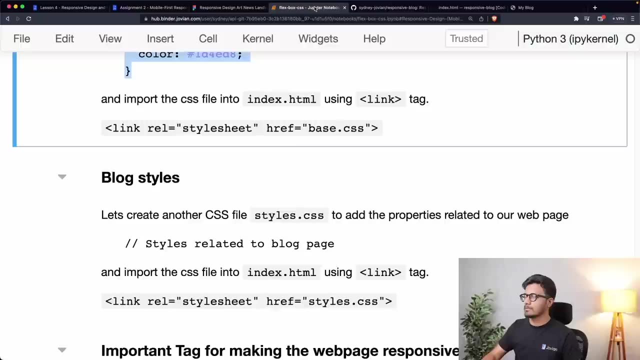 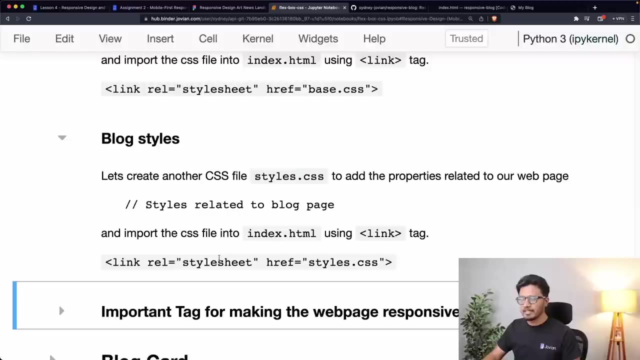 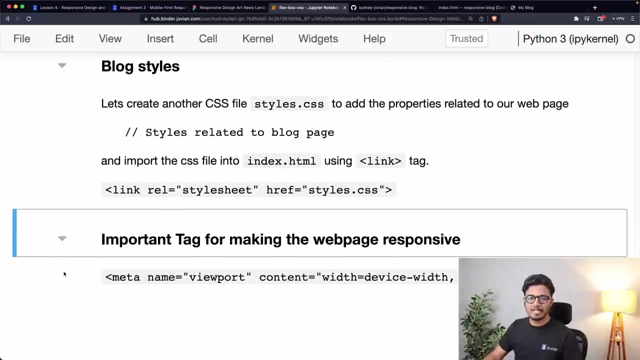 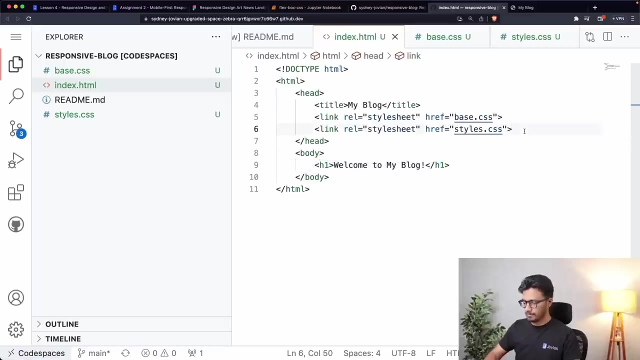 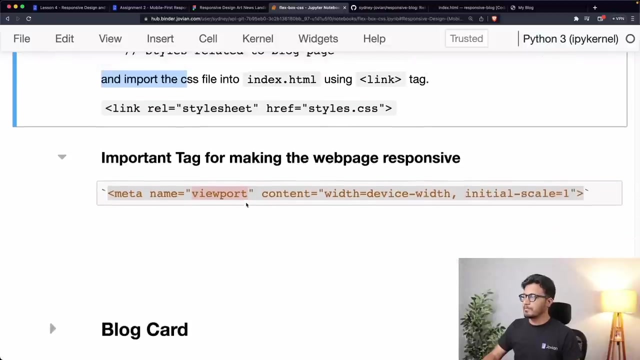 base dot CSS file. all right, you. so there is one more important tag that is required to make our web page responsive, and that tag is the meta tag, which has the proper attribute of name viewport. so we also need to add this to the head tag right now. thank you, agree, okay, so now we're set up with our environment and 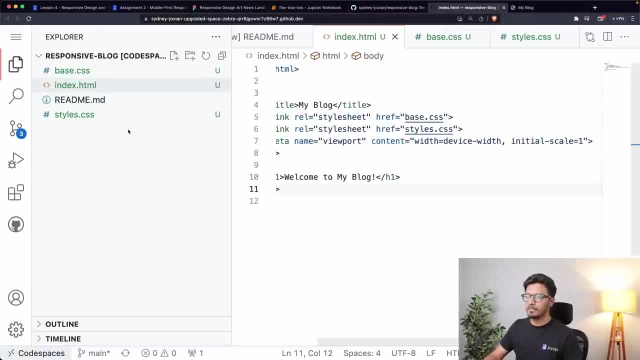 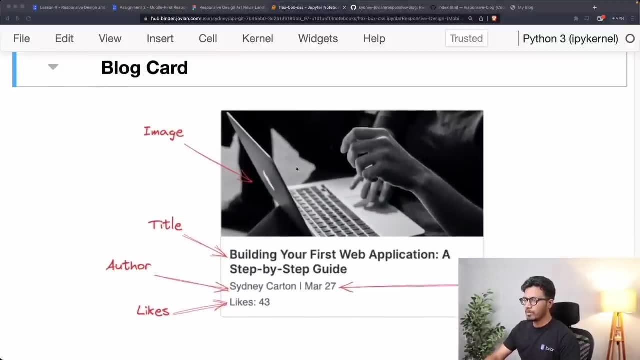 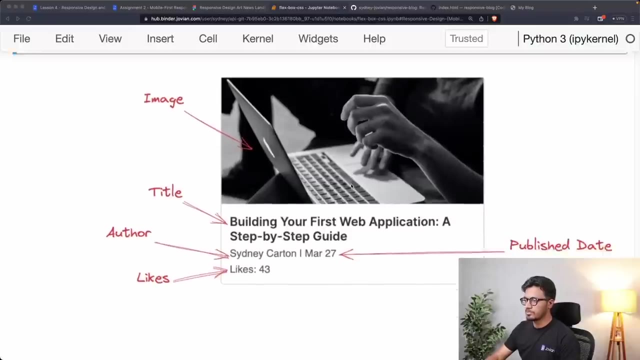 basic HTML and the files which we will be working on today. so the basic area of today' mock-up is this blockart which is going to be consistent across all the layouts we have seen in the mockup. so inside this blockart, theasing is placed inside our 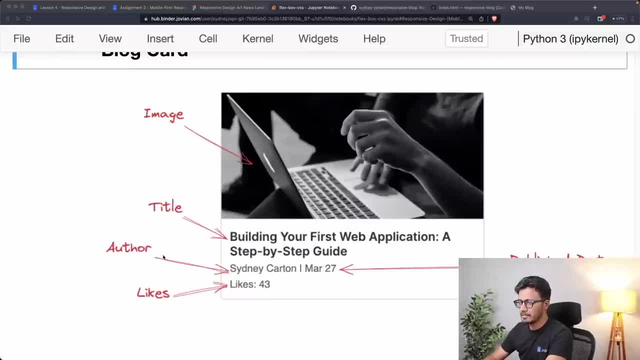 we can see that there is one image, one title, author, publish date and likes, and i am able to see that there is some spacing around the content, so maybe i will have to use some padding left and that needs to be applied to all the content. so that is one way, other way. 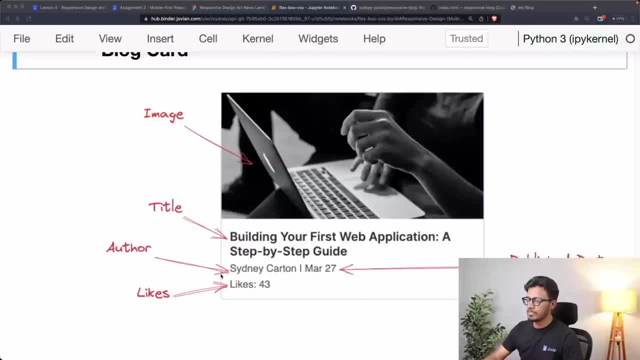 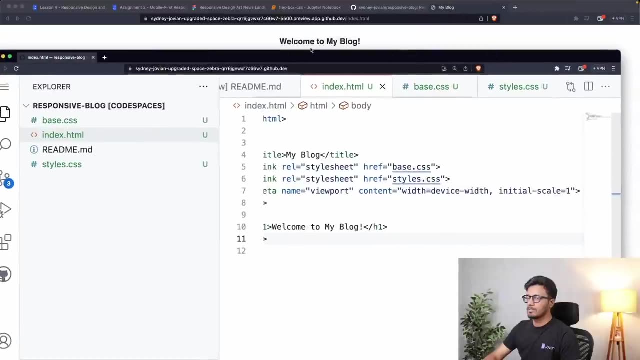 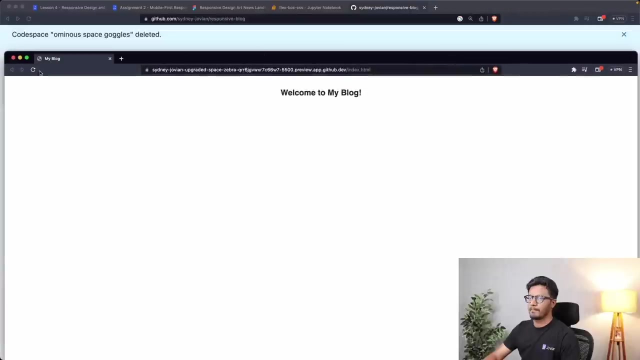 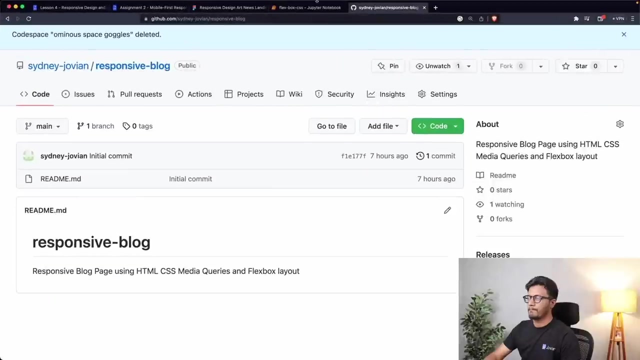 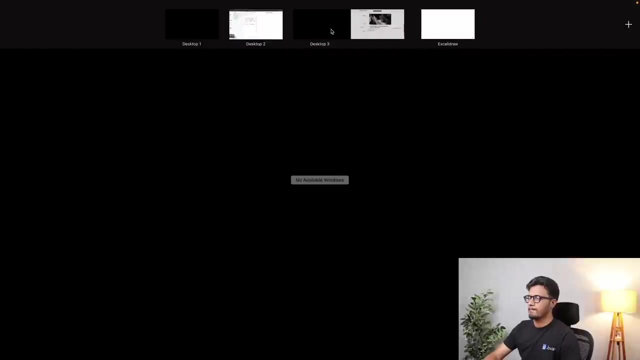 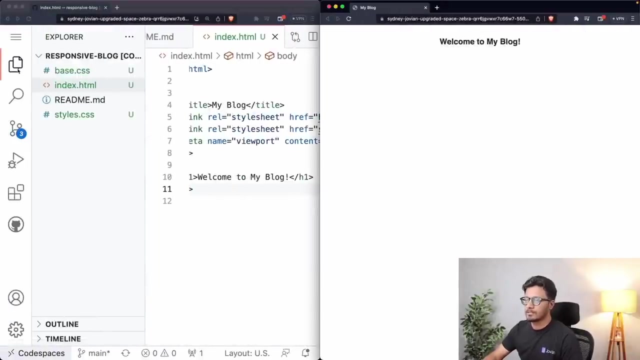 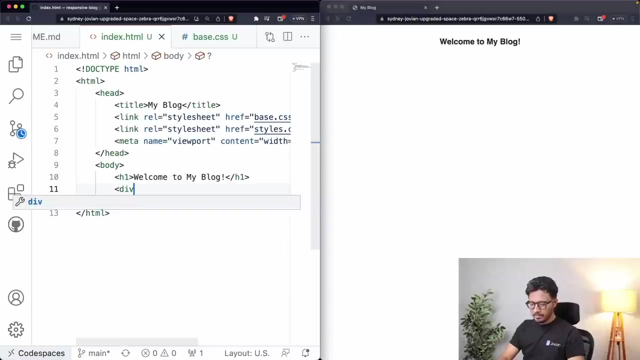 i could think of this is adding one outer div which will contain the title, author and likes. so let's add this html code. let me quickly resize this a bit, all right, so let's add a div which will be our div for the block card, and inside this block card you will require one div. 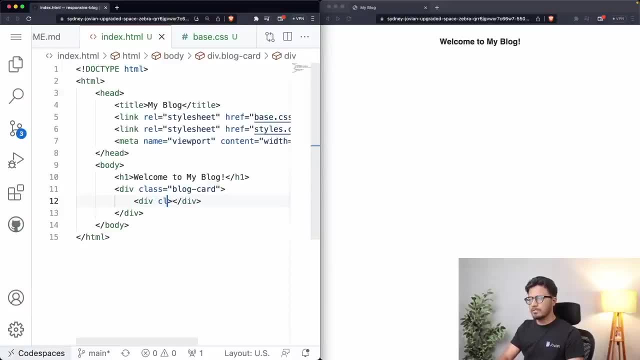 which will have the image for our blog and for the title. we can use the div also, but i will use it as a restoration step. use h2 because it is the second prior title after the page title, so I will give it a class. 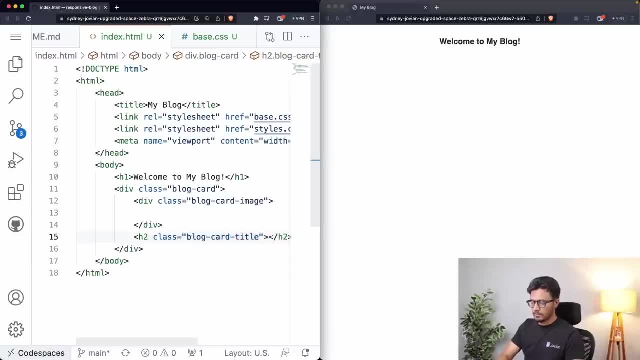 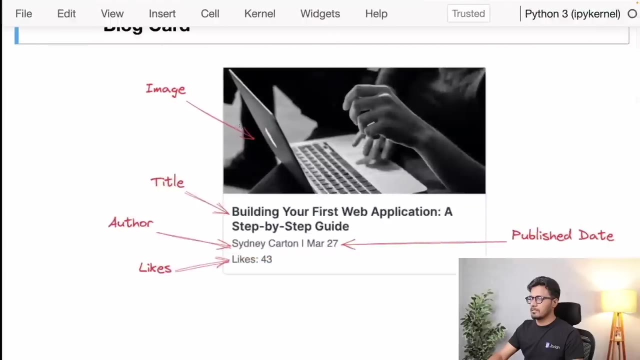 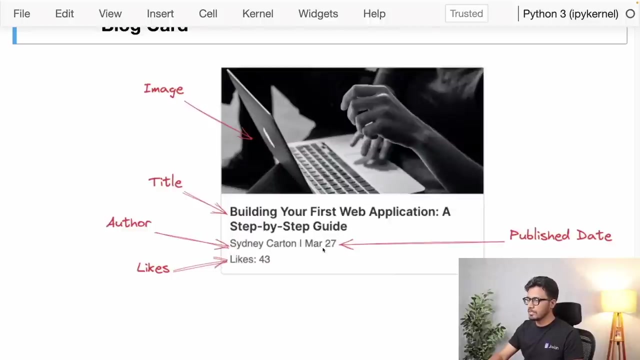 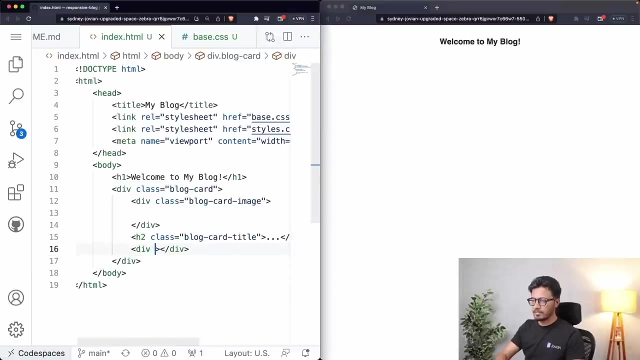 name: block card title. we will fill in the data shortly and after the title we have the author and the publish date. so maybe we can put this information in a single div because it is horizontally aligned. so let me add a div for that to the class. block card info. 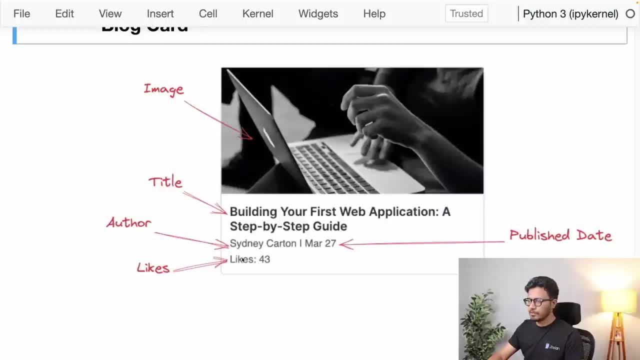 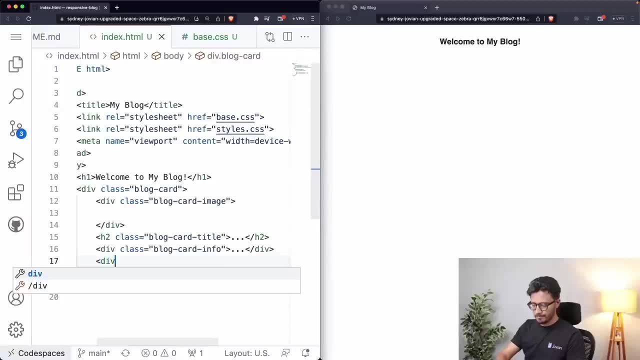 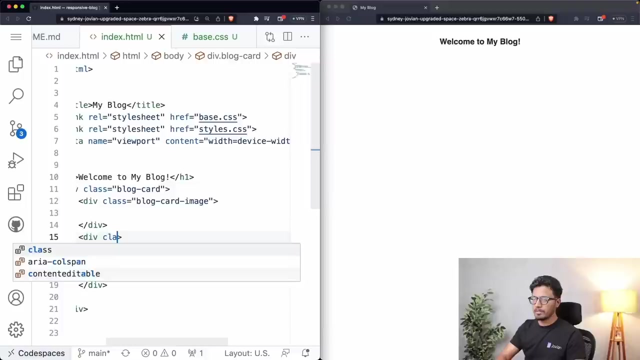 and one more div will be required for this likes count. all right, so we can wrap all these three elements inside one more div to add the spacing around them correctly. otherwise we will have to add the padding for each of these elements separately. so let's add a div and. 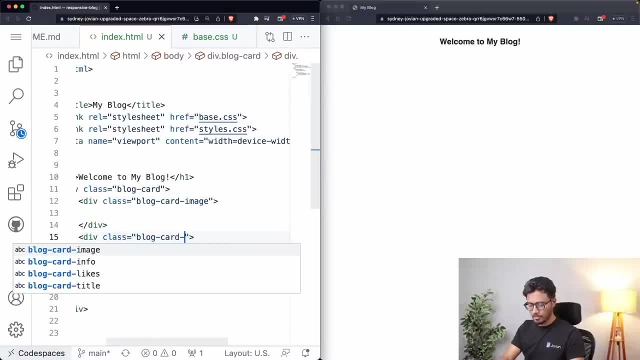 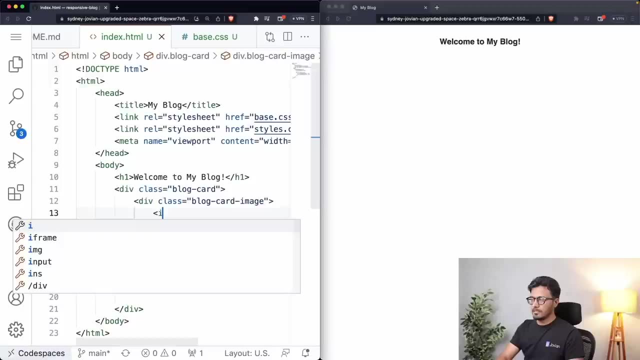 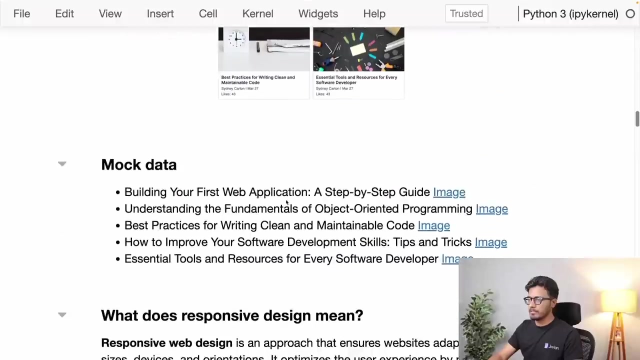 give it a class name, maybe block card body, and inside this image we will be having our image tag. so image tag has will have the src attribute and alternate text attribute. okay, so now let's put some data and see how it looks. so i will just copy the data and put it in the readme file so that we can. 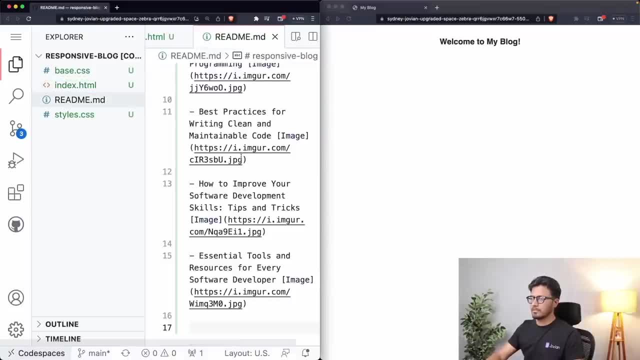 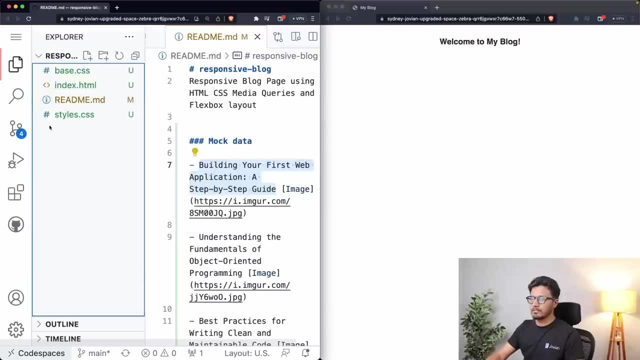 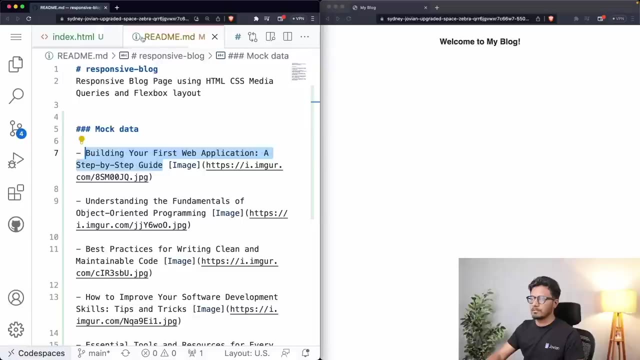 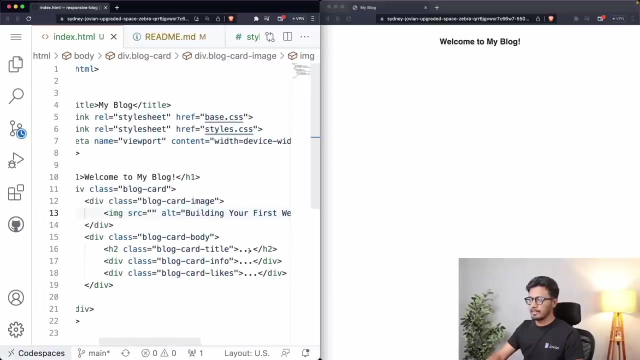 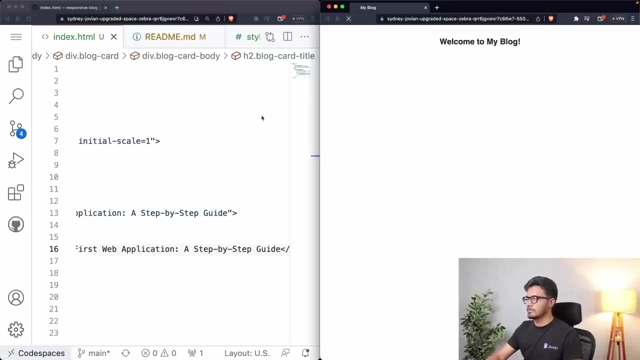 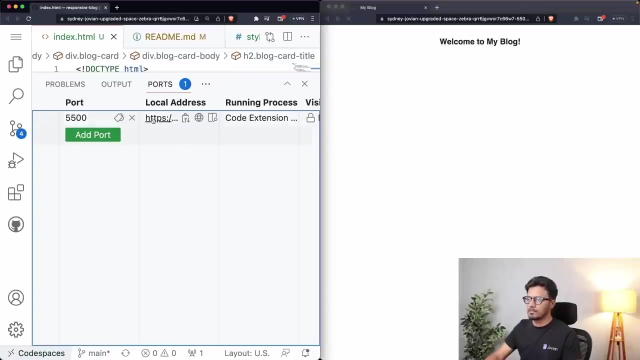 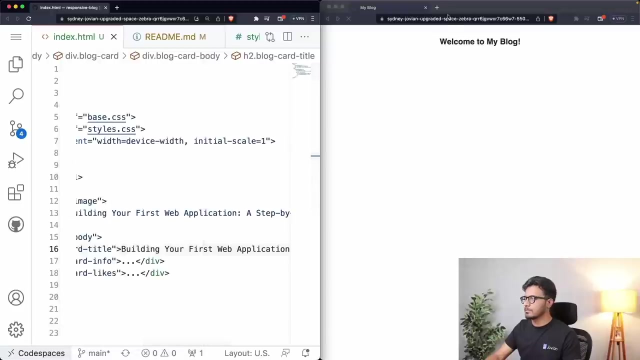 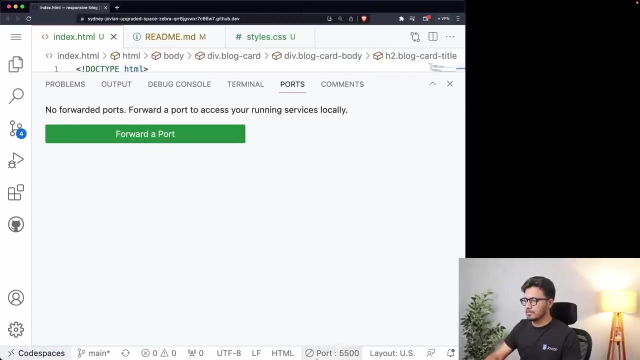 get it from here. let's copy the title first and put it in the alt tag as well as the title tag. let's refresh this once. sometimes it takes time. let me try to restart this. let me try to restart this. click, click, click, click, click, click, click. 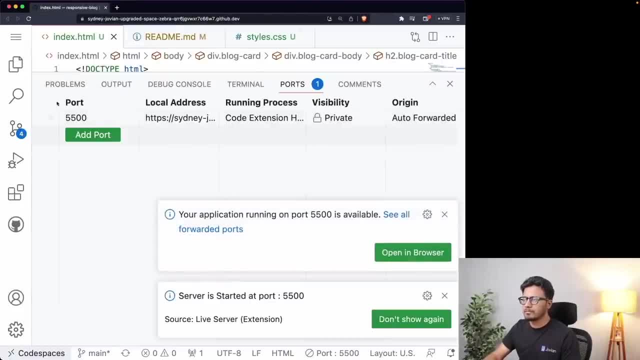 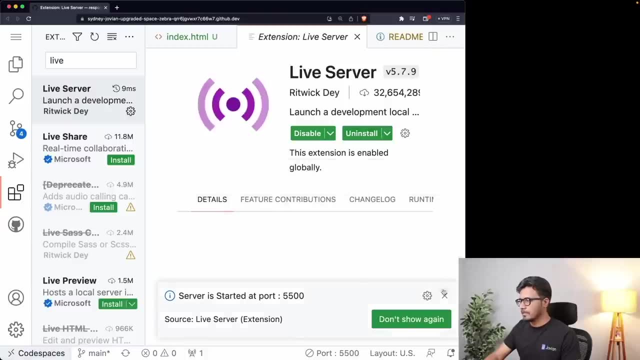 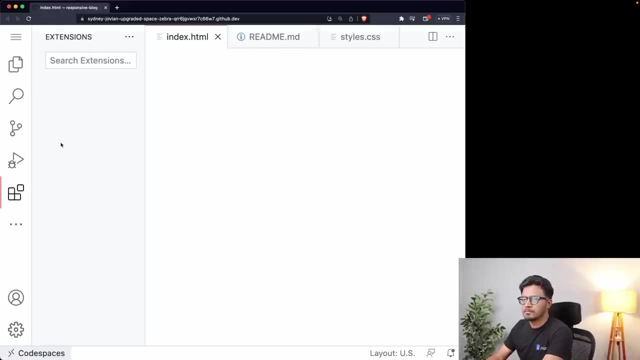 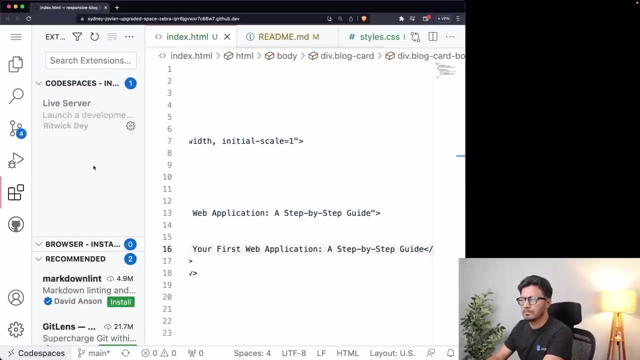 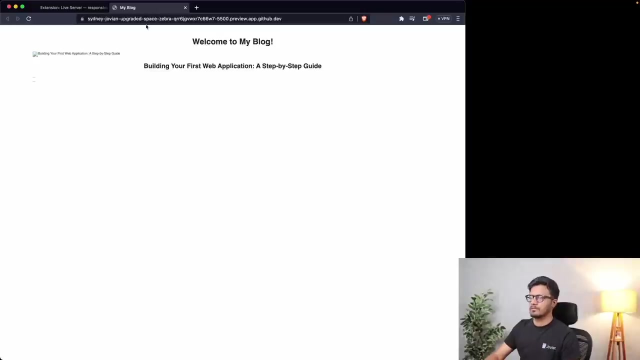 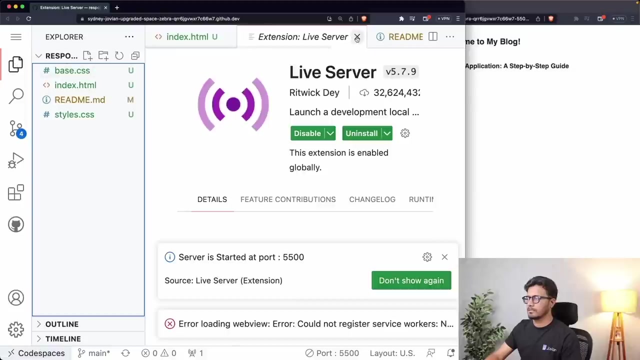 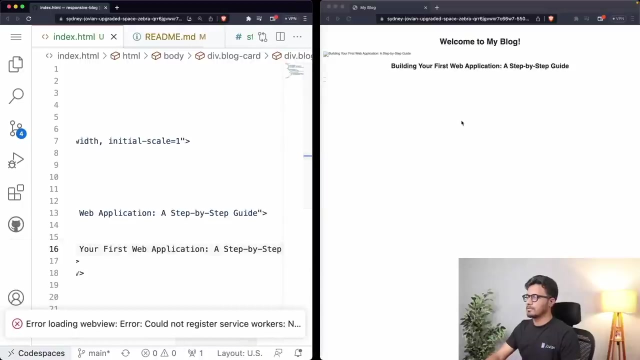 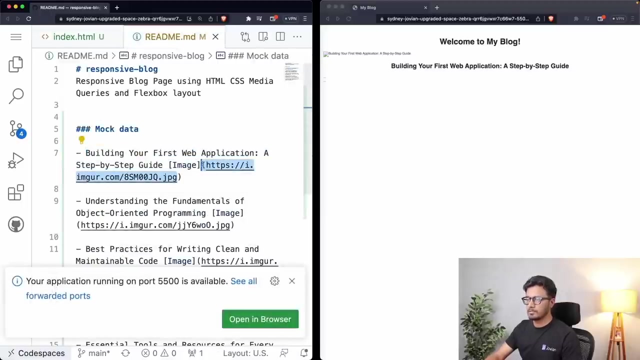 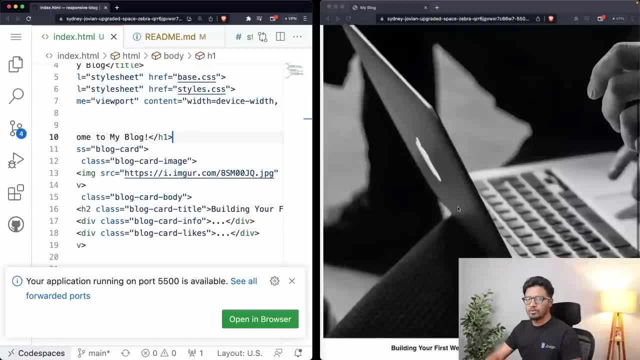 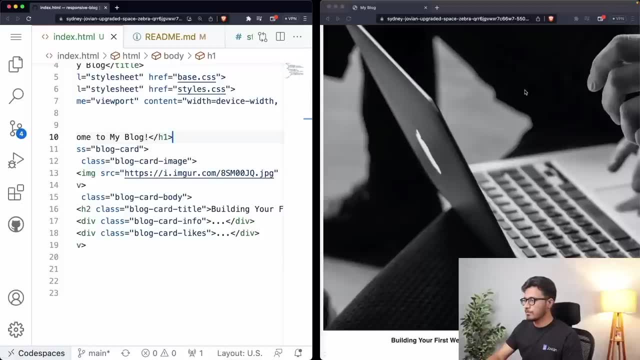 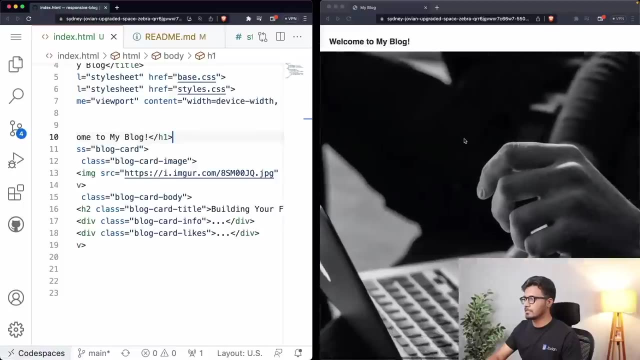 add that in the src, so the image is loaded and the title is also loaded, but we can see that we haven't added any property for the image, so it is taking its own width and height and it's maintaining its own aspect ratio and we can see. we discussed the key principle that the responsive design. 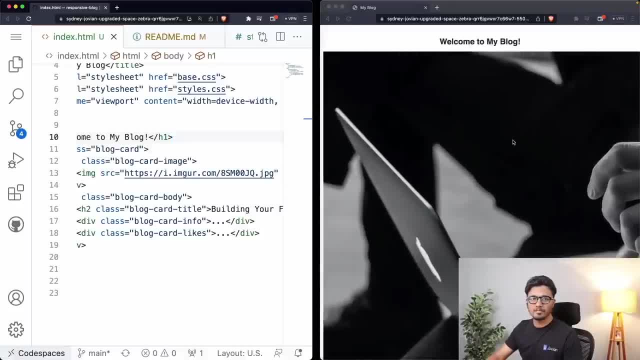 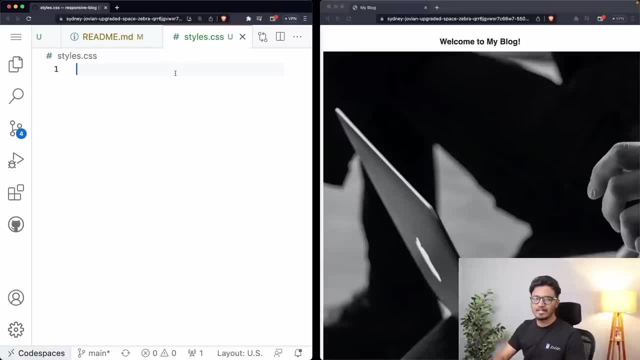 should not look like this, because we can see that the image is going out of the screen width. so for that we will need to add some styles. so let's create a style layout quickly. so first we have a block card, then we have a block card image. 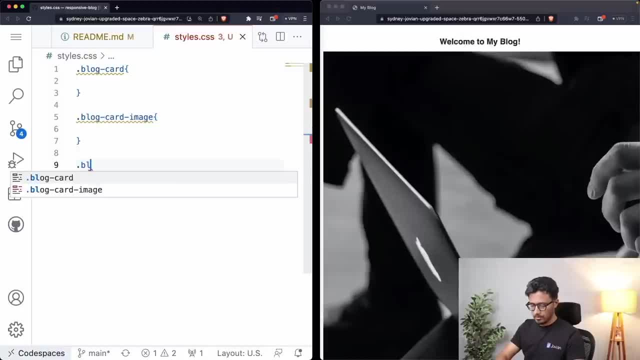 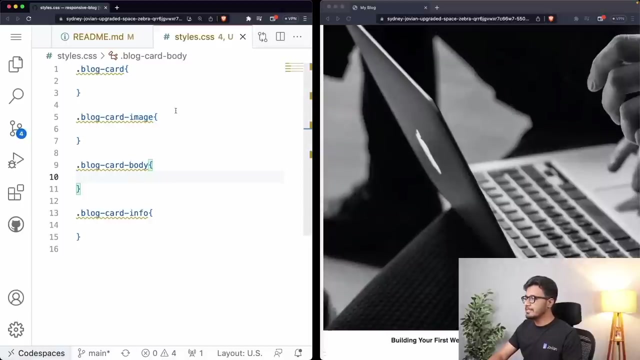 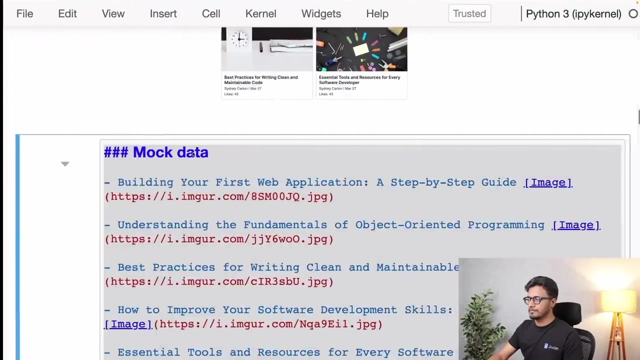 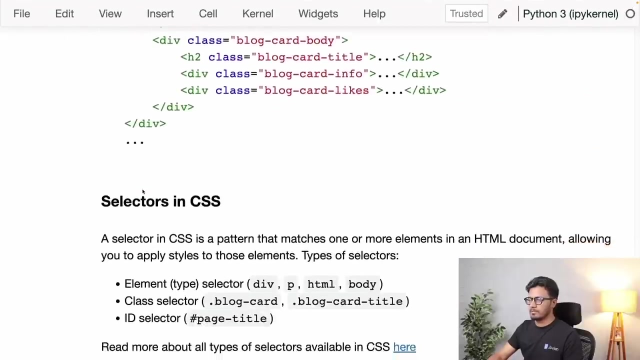 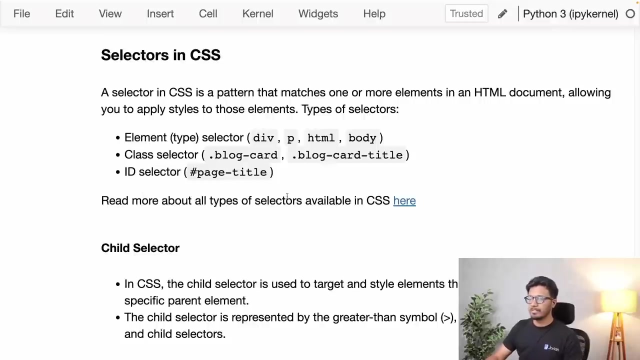 then we have block card body. inside this body we have one more div which is block card info. okay, so we'll need to resize this image correctly so that it doesn't go outside the screen width. so so for that we will be understanding the concept of selectors. so selectors in a css is a pattern. 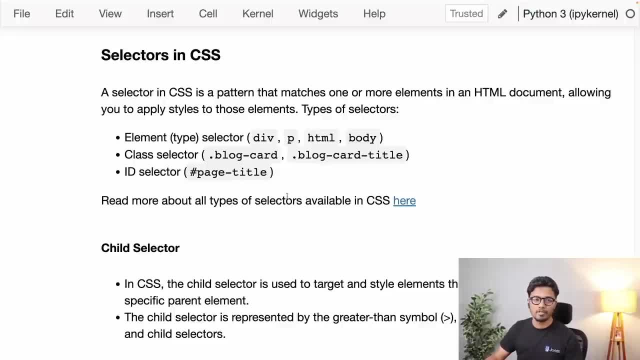 that matches one or more elements in a document, allowing your styles to apply to only those elements. so you have already used these selectors in your previous lectures and assignments. so the three basic types of selectors are the element selector, which applies to all the html elements, so div. 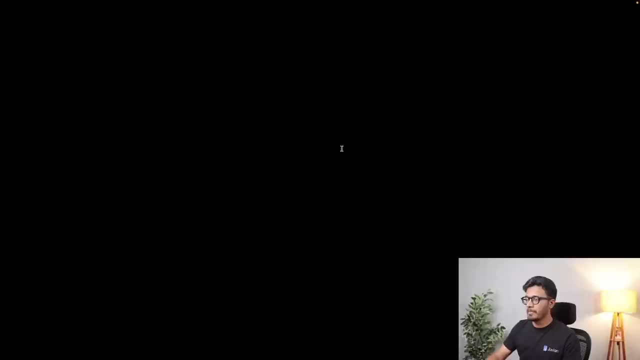 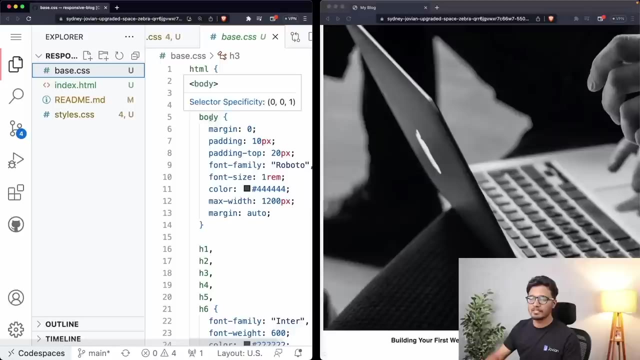 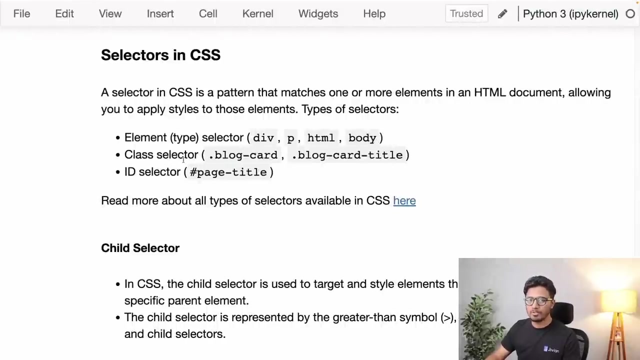 tag: html body. these are the elements. so in our basecss file we have used the element selector, so these are all the element selector and these styles are applied to these elements. next is the class selector that we are going to use in our stylescss file and third is the id. 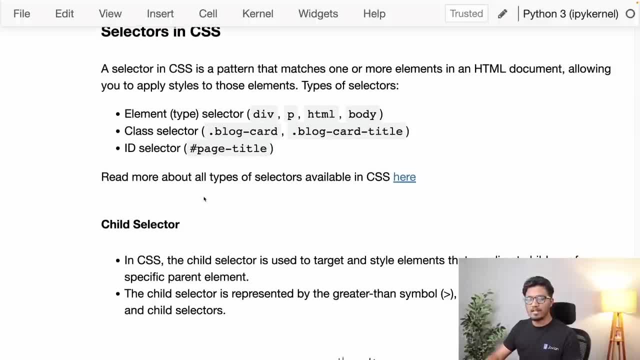 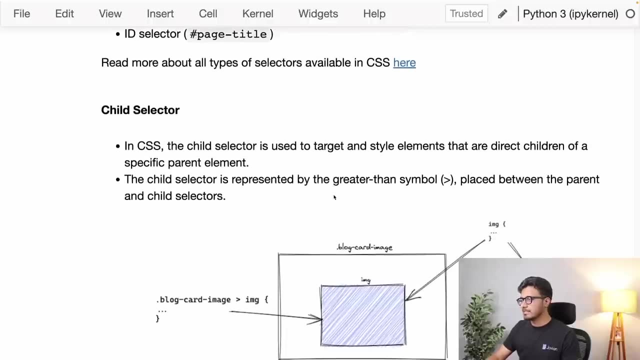 selector which begins with the hash. there are many more types of selectors in css. you can find it here. i have provided the link in the notebook. so the another type of selector is the child selector. so in child selector we have to specify two things. first, is the parent? 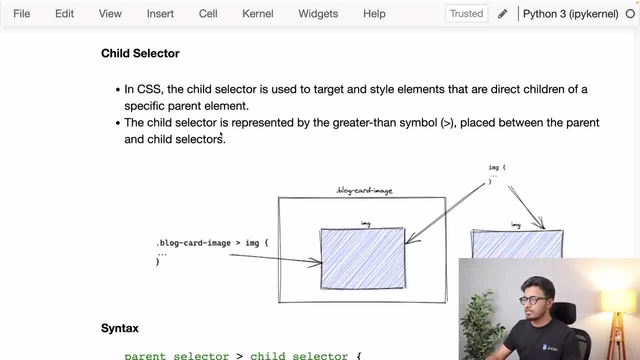 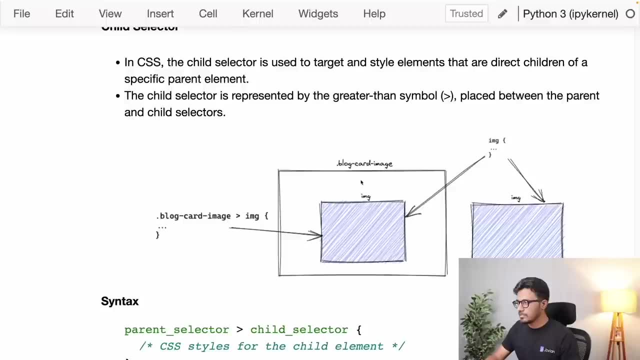 selector and the child selector. so that is specified using the greater than symbol. so let's try to understand this using this image. so in this image i have a div whose selector is greater than symbol and the time of the child selector. i have a div whose selector is greater than symbol and 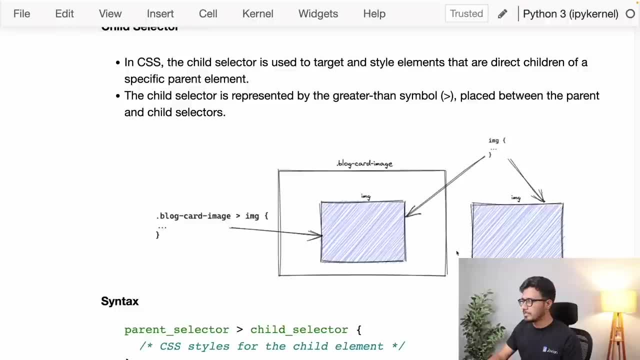 theender. going forward to this, we define css춰, etc. let's call this vest. imagine this of rank relationship with class, class elder, Which is inside a parent whose class is block card image. So for this particular use case we can use the child selector. 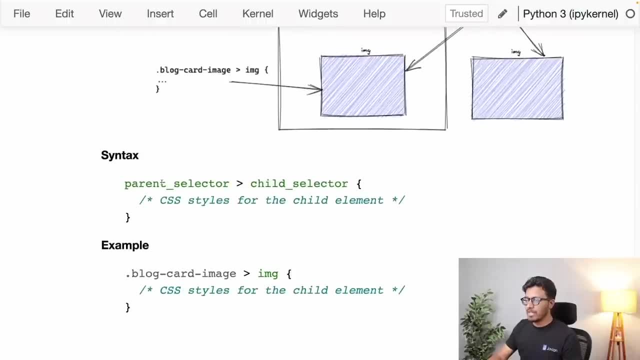 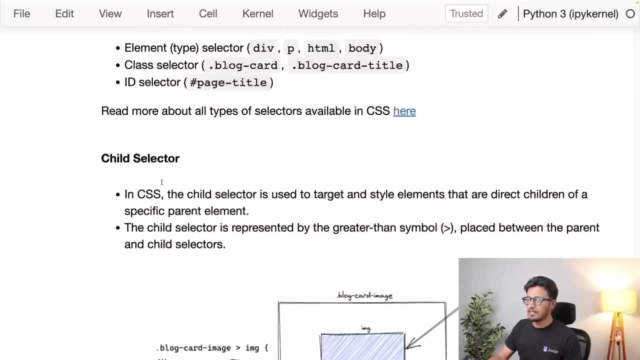 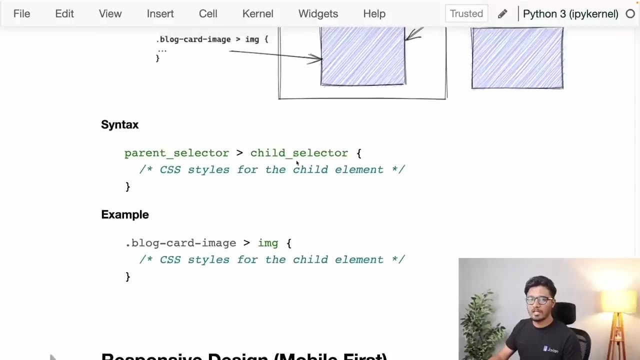 So the syntax for that looks like this: We have to specify the parent selector. It can be either ID selector or class selector or element selector, And same thing can be applied to the child selector. It can also be element, class or ID. 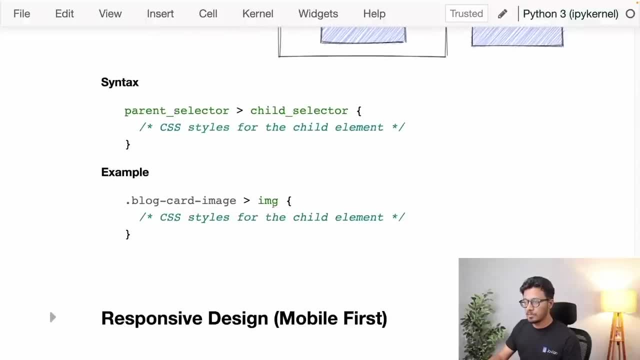 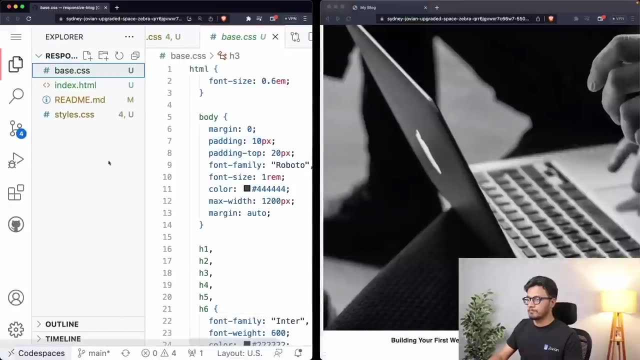 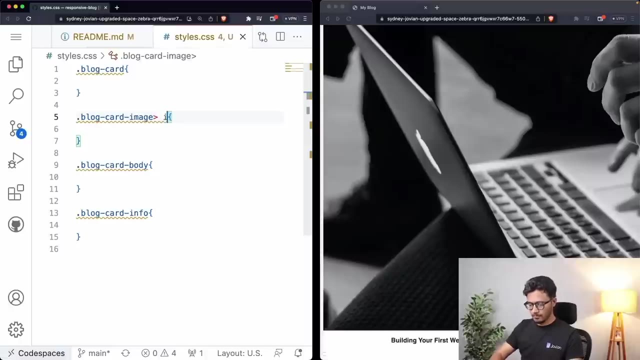 So we are going to use this to style our image. So we will be using block card image greater than image. So let's add that. So we will use the object fit property cover: Width 100% And height, let's say 160px. 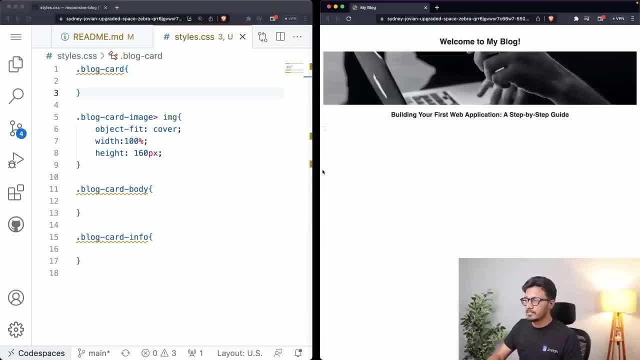 So we can see that the image is resized and it is not going outside our screen width. And also we can see that the image is not stretched. So we can see that the image is not stretched. So if you resize the window, you will see that it is getting scaled in and scaled out, but not getting stretched. 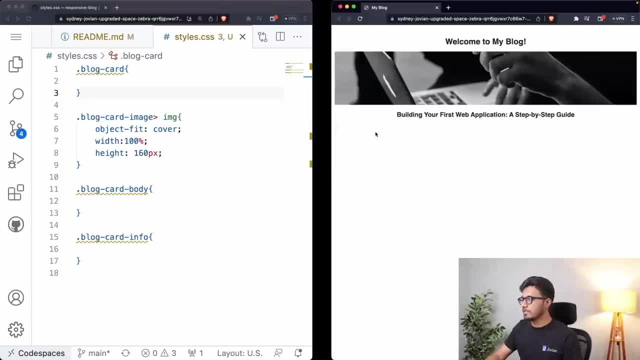 So this is how we want our HTML image to render in a particular screen width. So let's quickly add few more styles to our block card title. So let's quickly add few more styles to our block card title. We can left align the title. 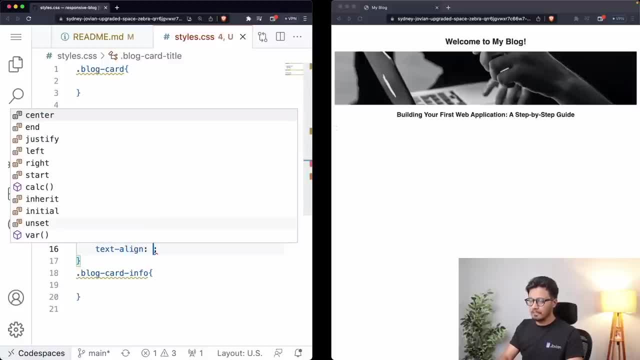 So for that we can use text align left And we can also reduce the font size a bit. That we can do using font size property, And let's make it 1.5rem. All right, And let's make it 1.5rem. 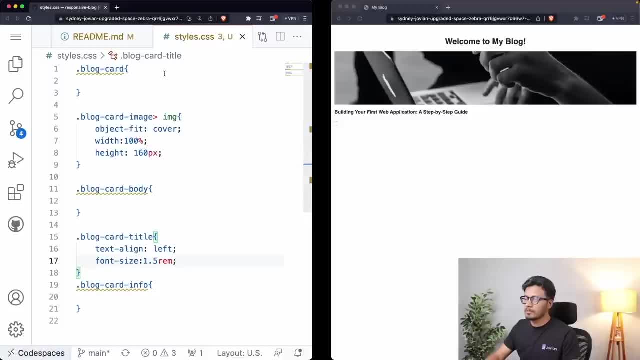 And let's make it 1.5rem. And let's make it 1.5rem. and now we can add some border to the block card, so that can be done using the shorthand property of border, whose first value is the width of the border. so we will keep it 1px. and then the style. 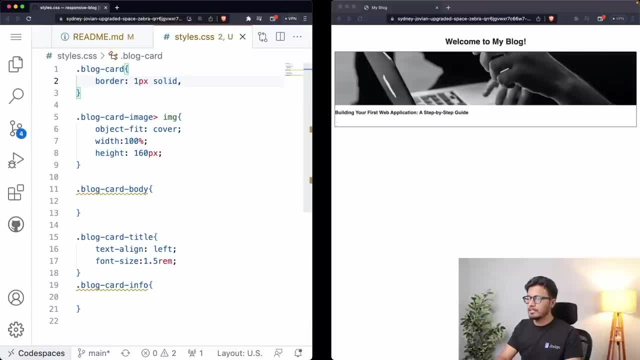 of the border, so we want the solid border. and the third is the color. so that can be any rgb color, so let's choose some light color. so fff stands for white, so something darker than white, maybe let's try ccc. yeah, so this is fine. 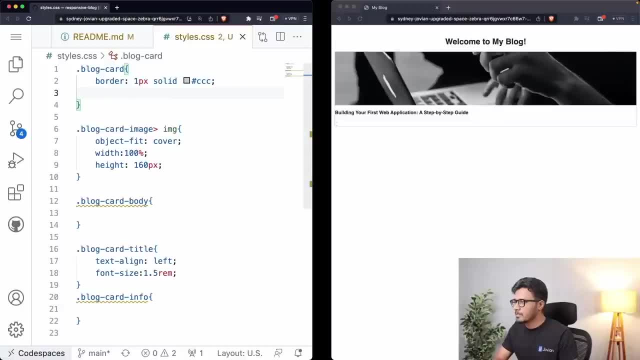 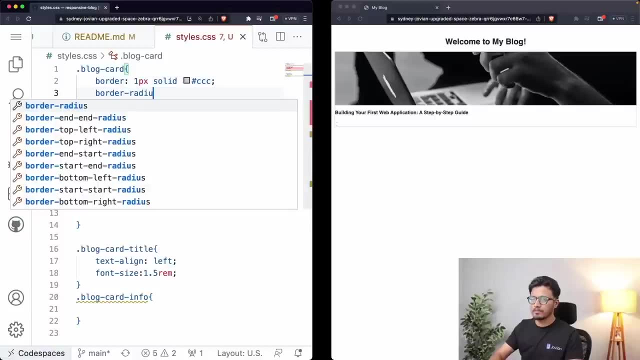 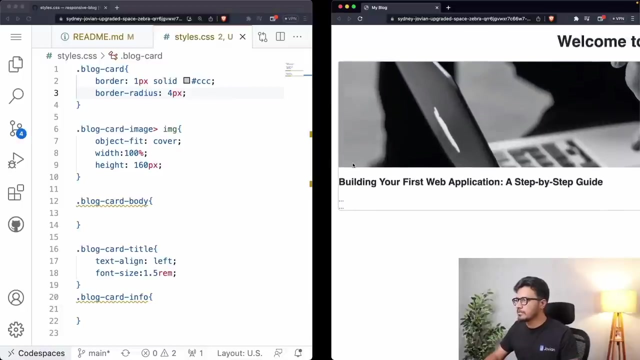 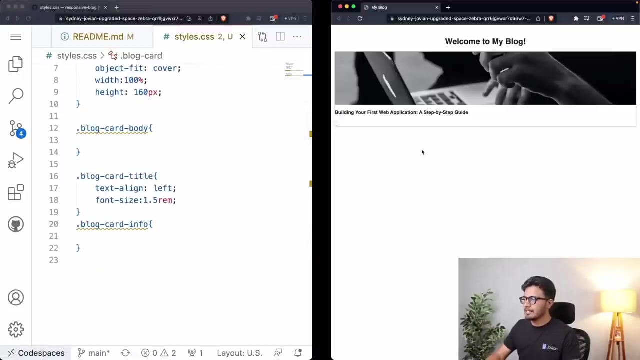 and also let's add some border radius to, let's say, 4px. all right, so we can see that the border and border radius are added to our block card. now we need to add some spacing here, but before adding that, let's also add the other. 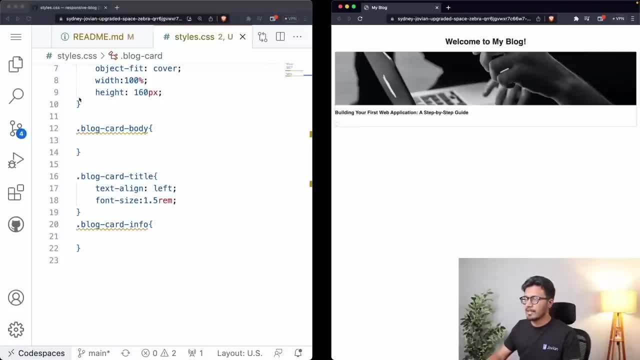 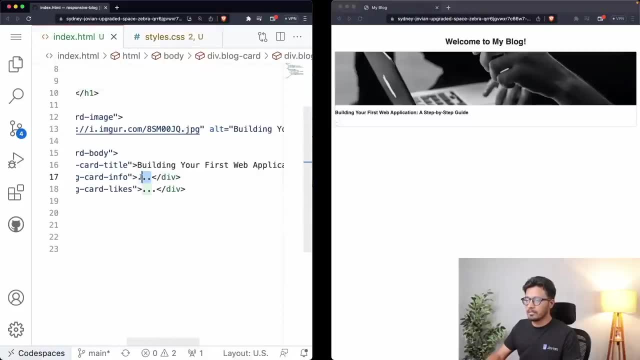 information of the block, the author and the published date and the likes count. so we can go here and we can add some spacing here and add the author name, carton and, let's say, the publish date. you can put today's date and the likes to be, let's say, any random number, 256, okay, yeah, so the content for. 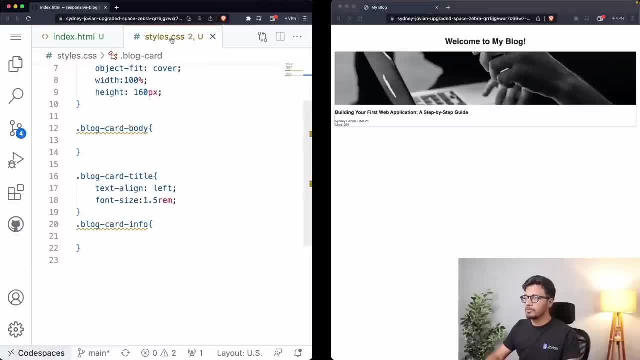 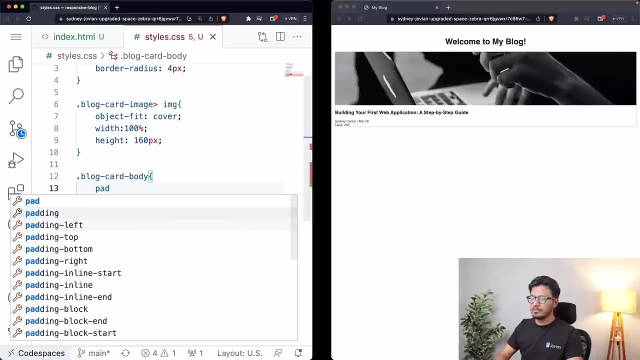 our block card is the same as the other block card, so let's add some spacing here and add the author name and the likes to be, let's say, any random number, 256, okay, yeah, so the content for our block card- and add the author name and the likes to be, let's say, any random numberína. 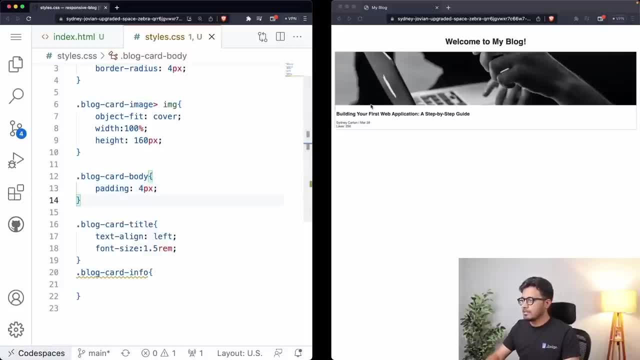 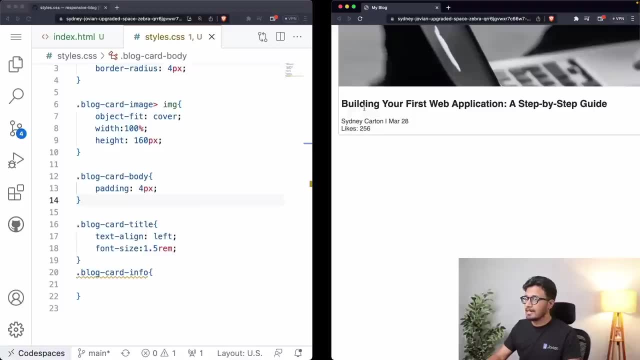 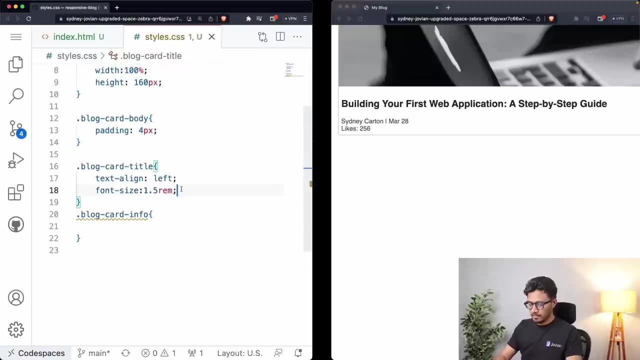 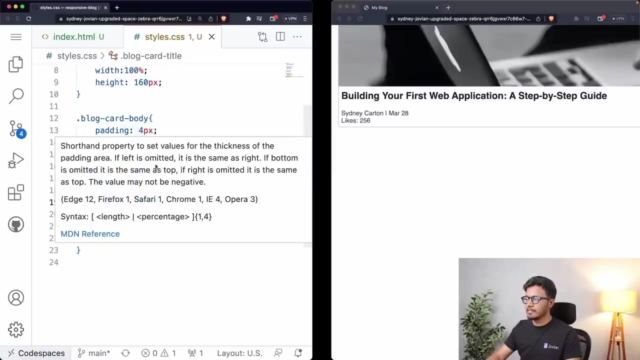 And we can see that there is a lot of space at the top of this title And that is coming because of the H2 tag that we have used. So we can reduce that. Maybe let's make it zero, because we already have a padding here. 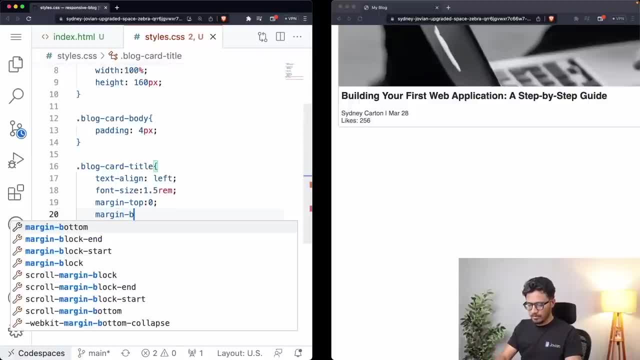 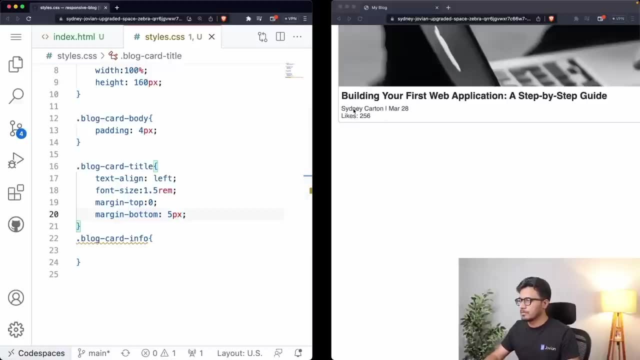 And also let's change the bottom to, let's say, 5px so that it's look more visually appealing, And we'll also need to add some spacing between the author and the likes to the author and the publish date. information is stored in the div which is having a selector block card. 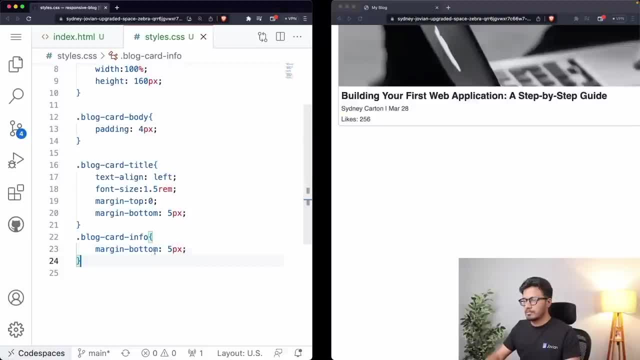 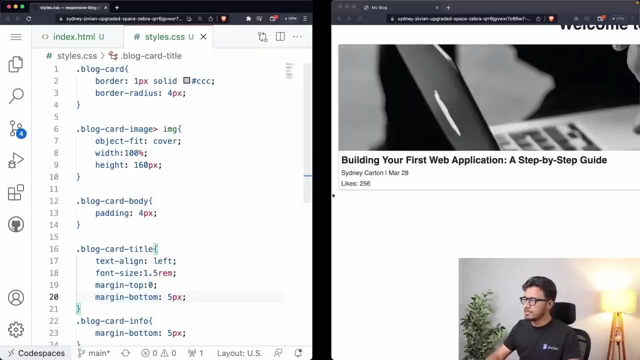 info. So we will add a 5px margin bottom to the this div. So now it is looking fine. Maybe we can increase the font size a bit, But we want a font size which is larger than the current one but less than the title of. 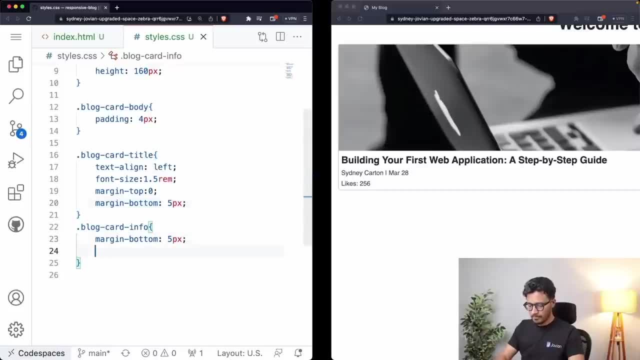 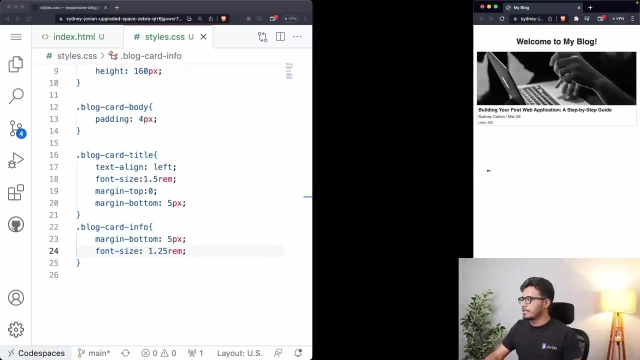 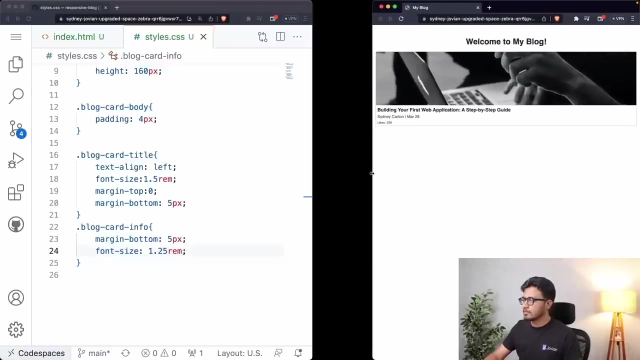 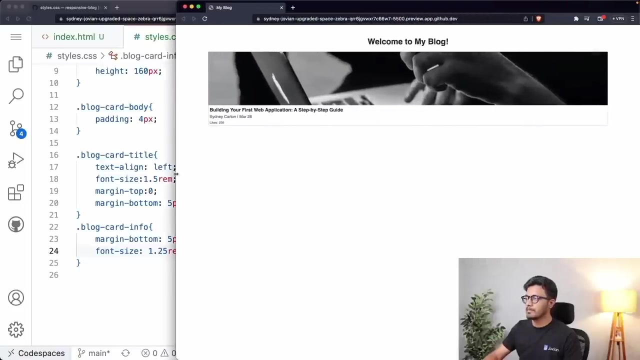 the blog- So let's try- is 1.25.. All right, so our block card is ready. Now we will have to make it like. we will have to set the max width, because we can see that it is getting scaled horizontally as I am increasing the screen width. but we want to. 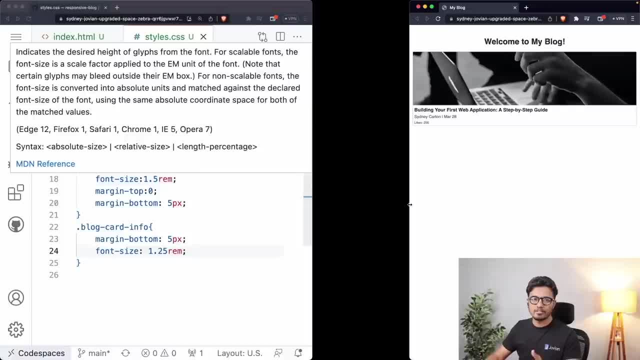 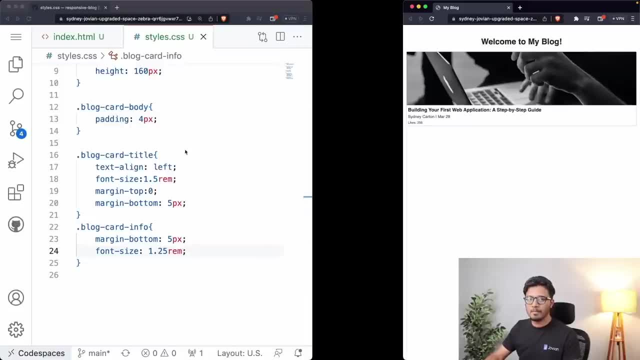 scale it up to a particular Width and after that it should have a fixed width. For that we will have to add a layout that is the parent component to this block card, because right now it is taking the width which is available to it, that is, 100% of the screen. 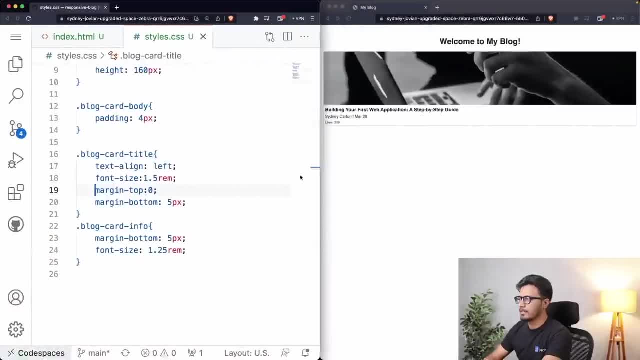 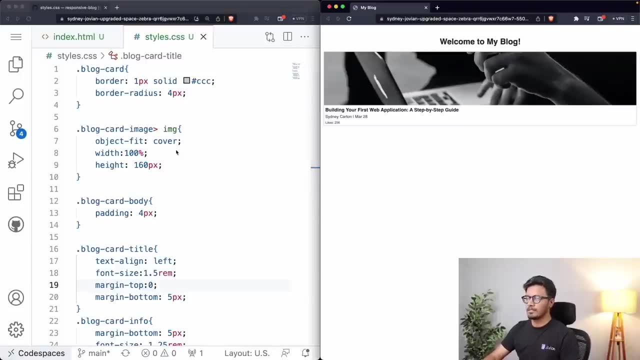 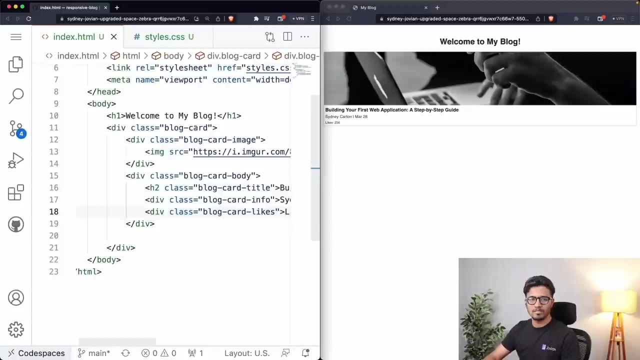 So we have designed the block card and it is currently looking like this. So now we will need to add some layout to this card. right now, As you can see in the HTML file, we haven't added any parent div to this card, So let's quickly add that. 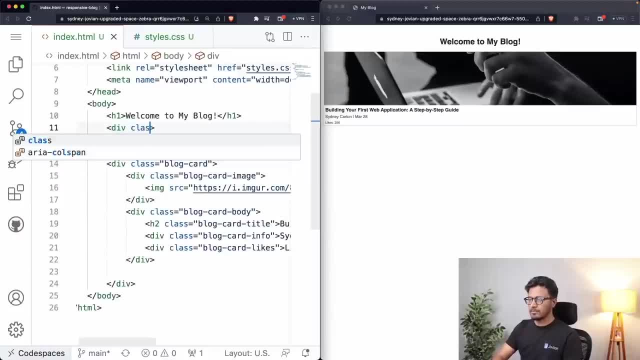 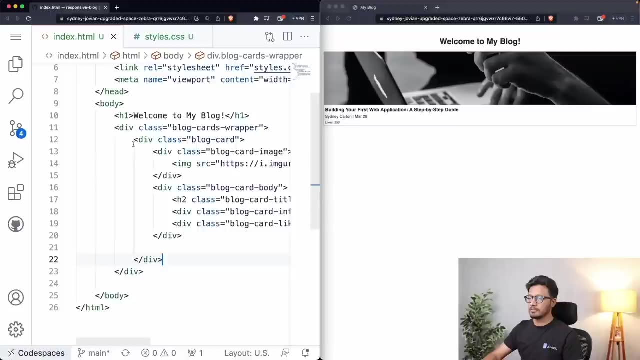 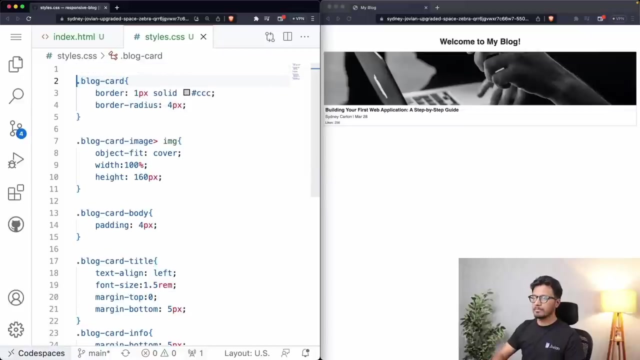 I will create one more div whose class name we can call block cards wrapper, And we will put this block card inside this, And let's define some file for this block cards wrapper. So I don't want the block card to take the complete width of which is hundred percent. 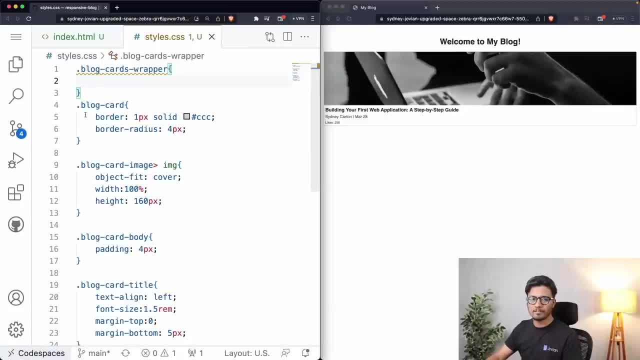 So it should scale up to a certain limit, but after that it should have a fixed width. So for that I will have to use a max width property, And so we are designing for the mobile view first, and mobile view, the max width is 576. 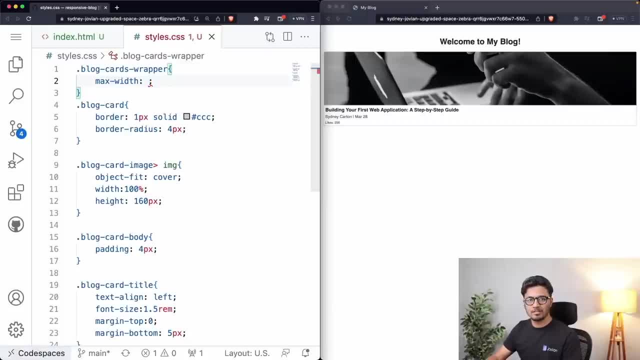 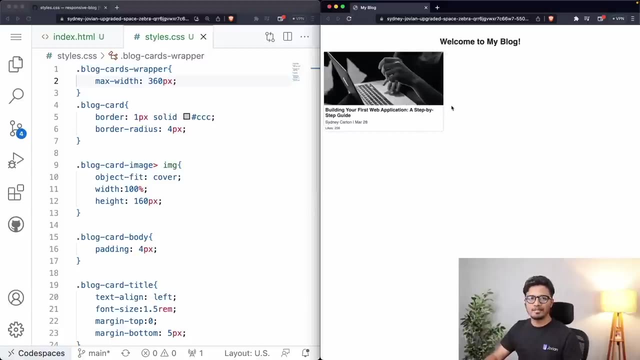 px, So our max width should be such that it is less than 576.. So I will just use 360 px And refresh the page. So now you can see that the block card is restricted by its parent component or elements max width, which is 360 px. 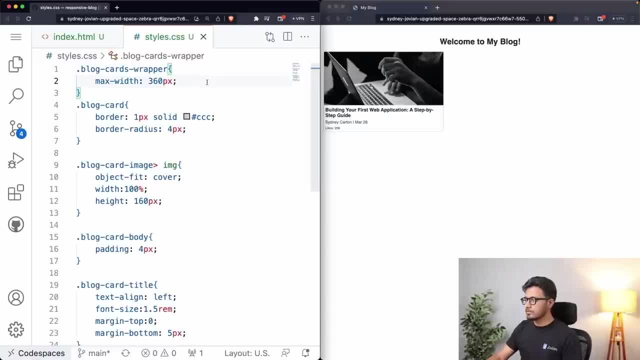 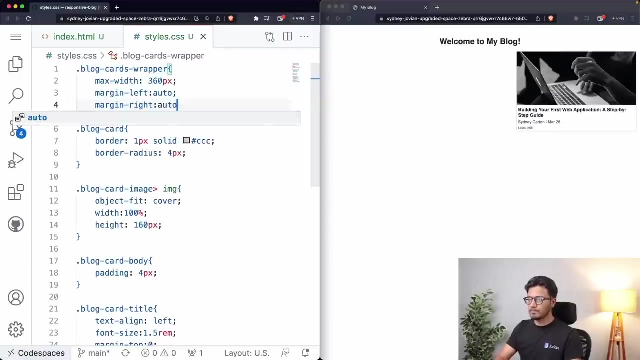 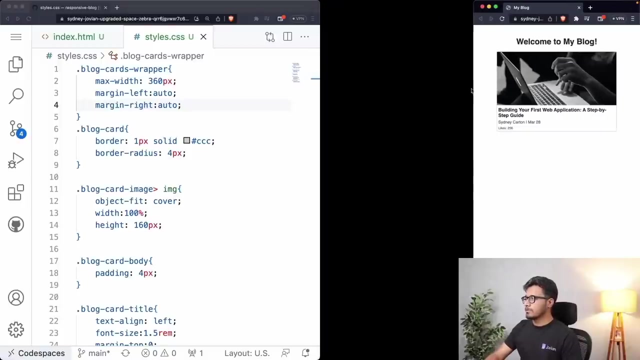 And also, I want all the blocks to appear centered horizontally. For that we can use margin left auto. It will auto center the block cards wrapper horizontally center. Okay, So now let's see the device more quickly. Okay, So now let's see the device more quickly. 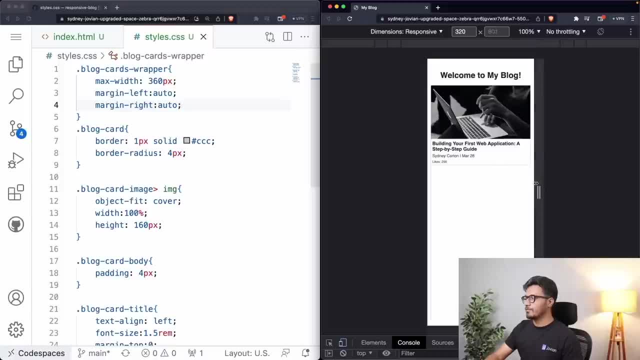 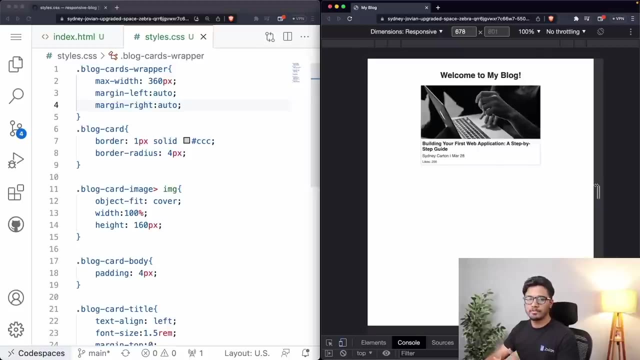 And if we go to 320, you can see that the card is scaling up to certain limit in 360 px And then it will be a fixed width. In this way we are restricting the card width so that it looks consistent on all the devices. 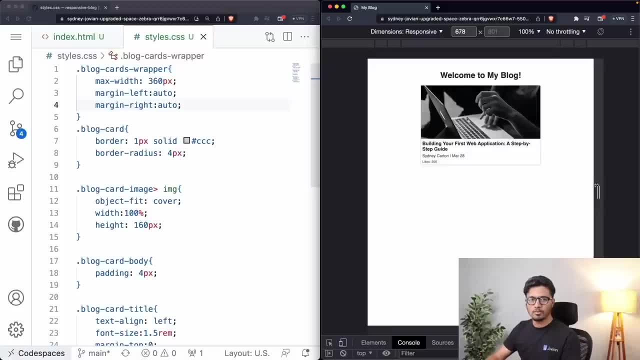 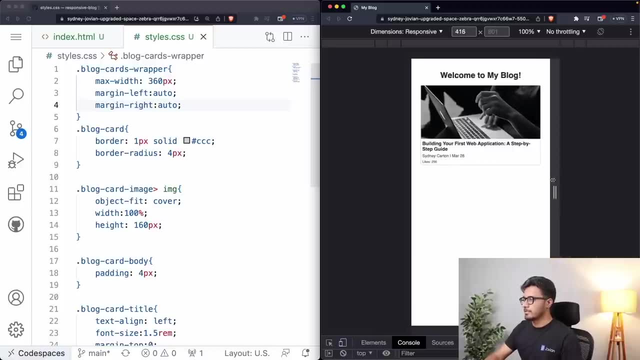 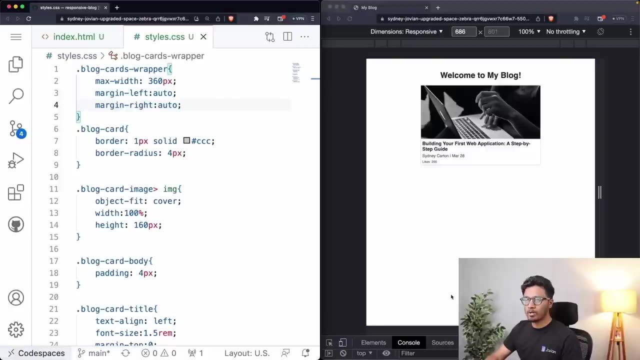 because we are working for a range of devices. All devices might have different width, So The page might not look consistent, So let's So. that's. that is the importance of adding the max width to the wrapper. So now let's add a few more block cards to see how the vertical layout looks like. 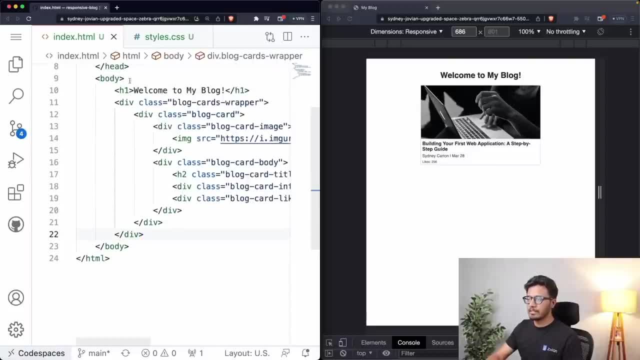 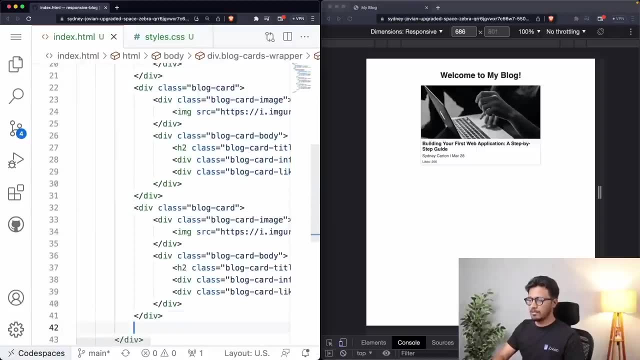 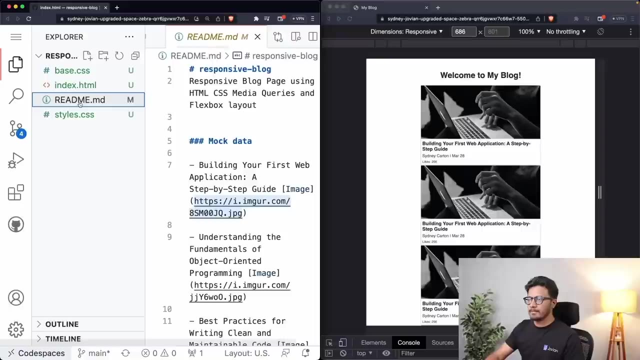 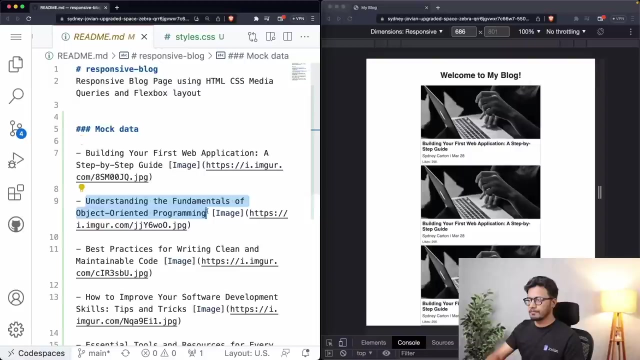 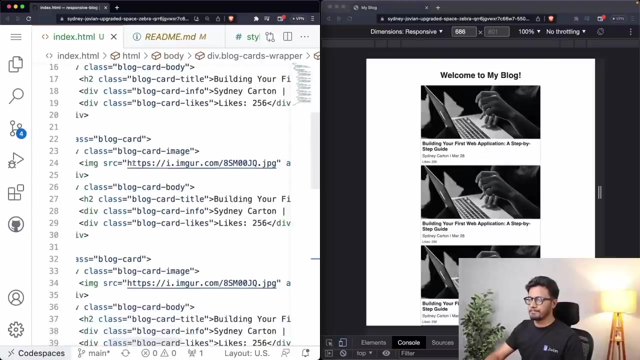 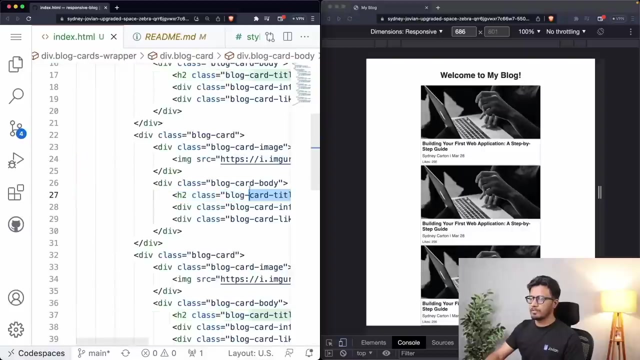 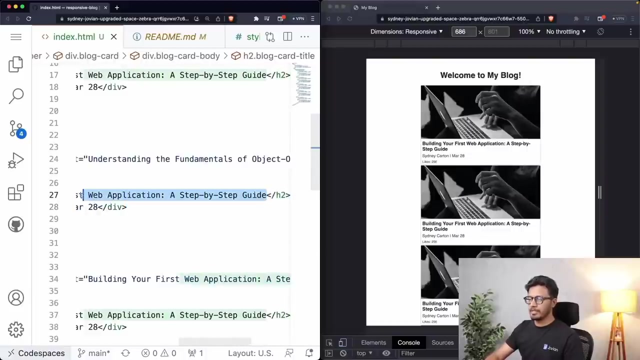 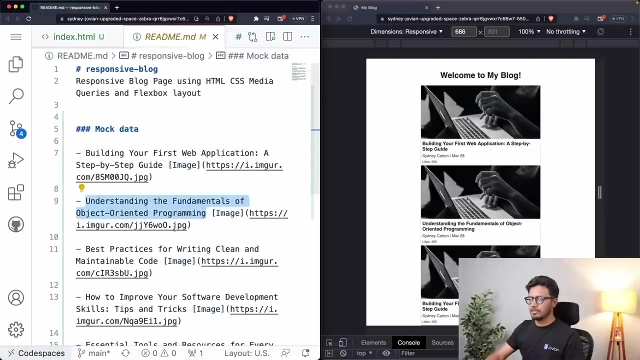 For that we will need some more data, and let me quickly see these types And grab the mock data from here. We will be adding it at two places. One is the Image Alternative text attribute and other is the block title. And also let's add the image. 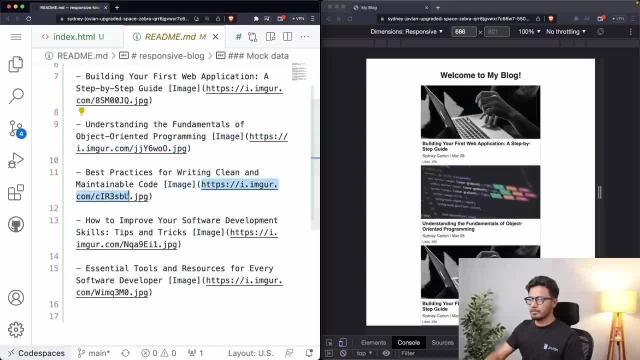 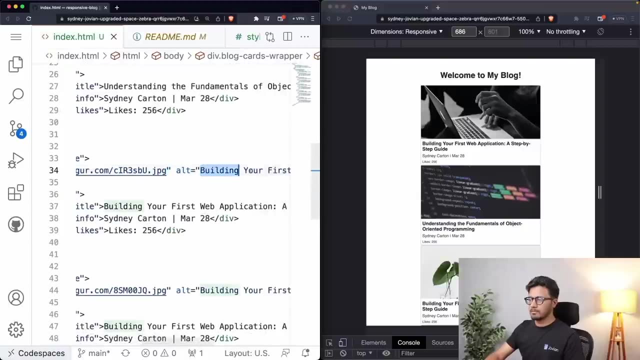 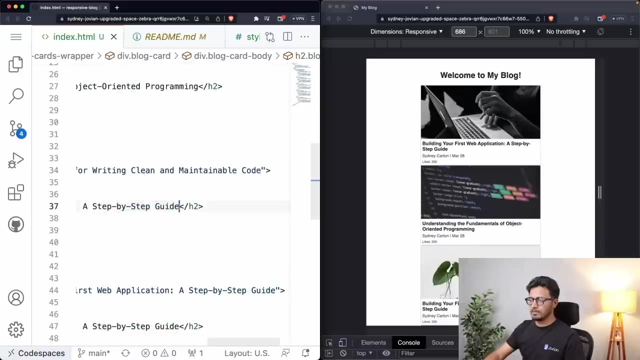 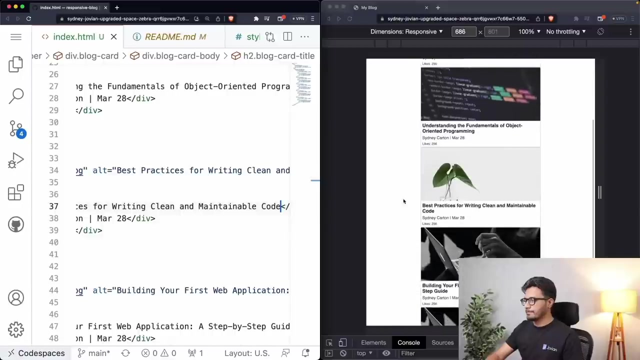 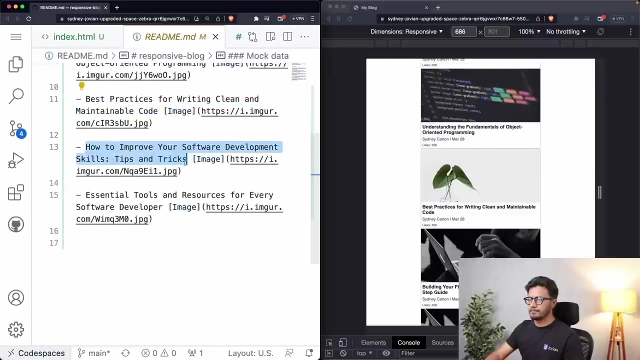 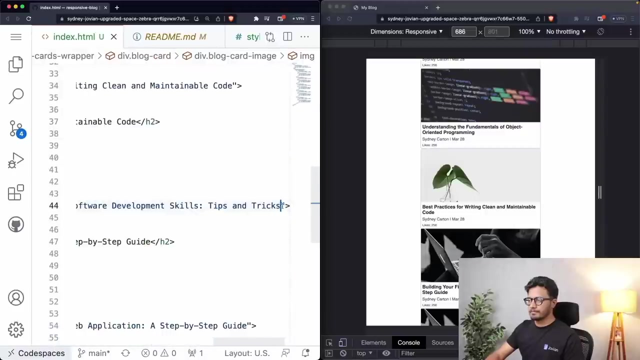 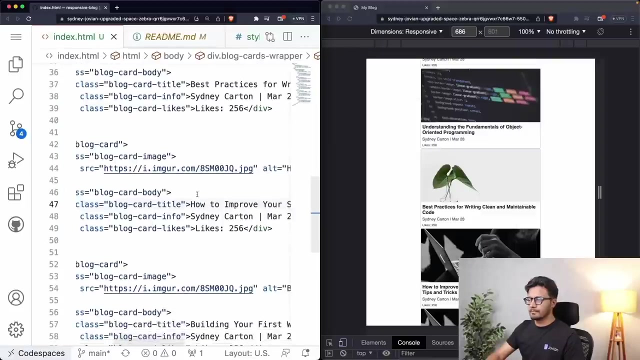 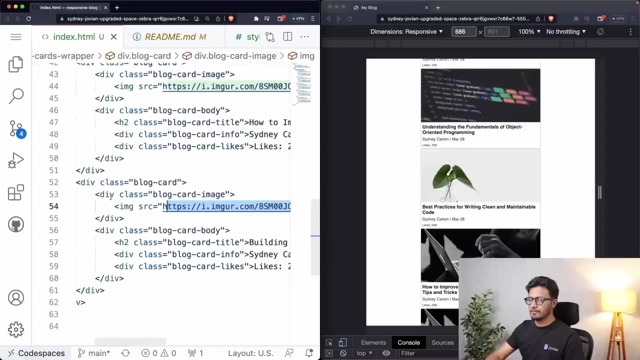 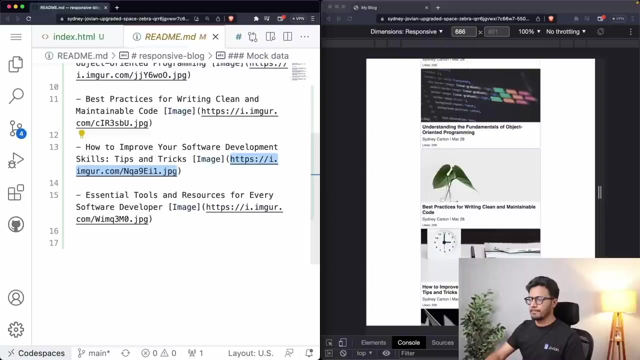 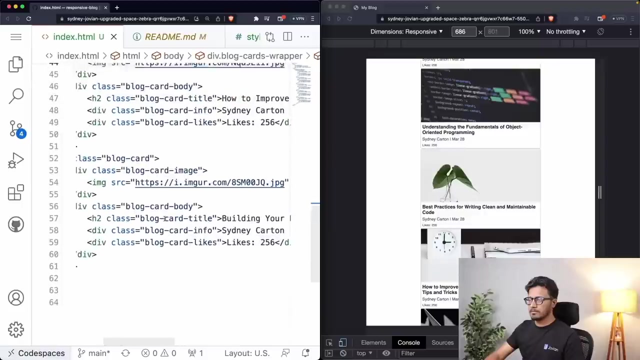 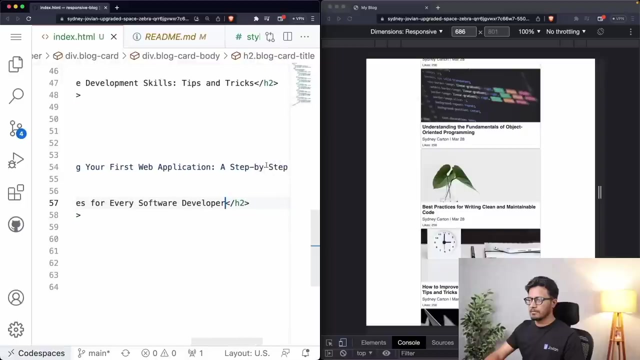 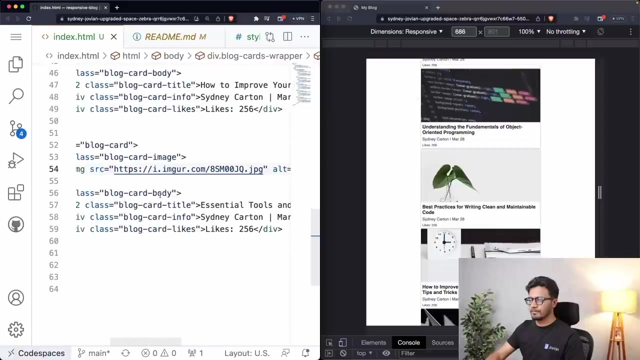 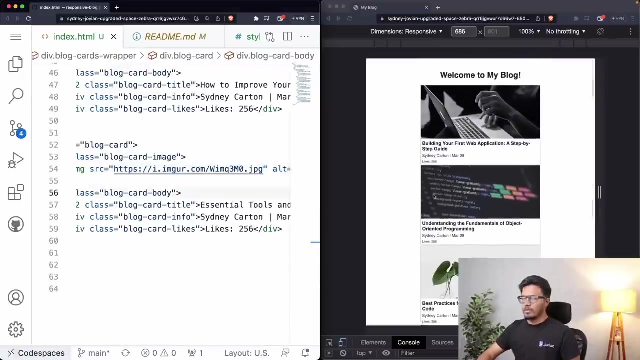 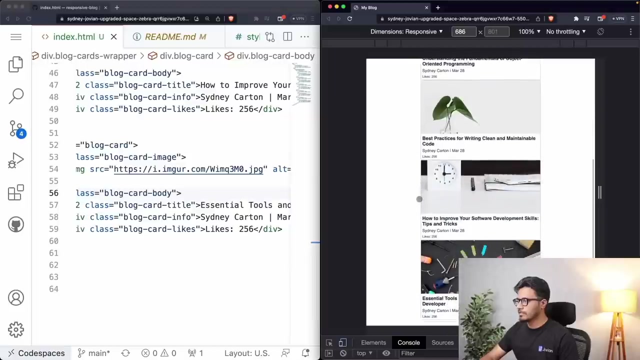 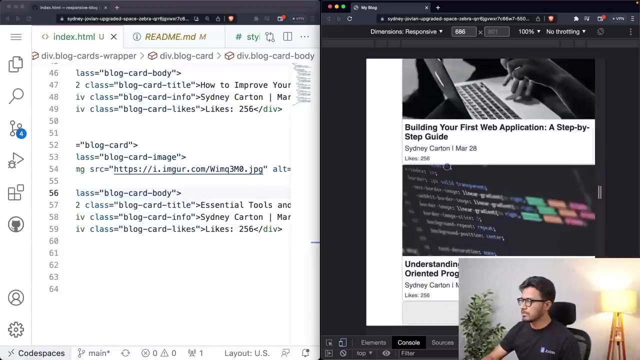 Loaded Other images Title: All right, so we have all the data in place and we can see that all the images and the title are loaded correctly. So We We want some spacing between two consecutive cards. right now There is no spacing. 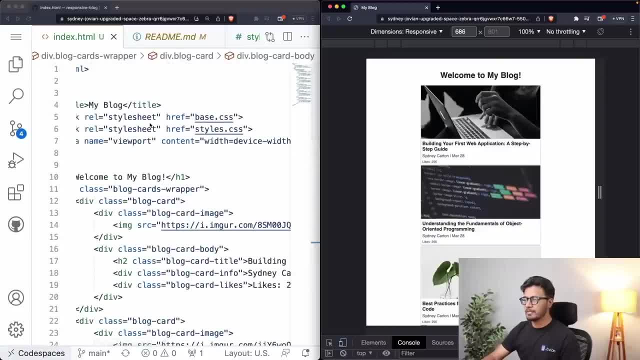 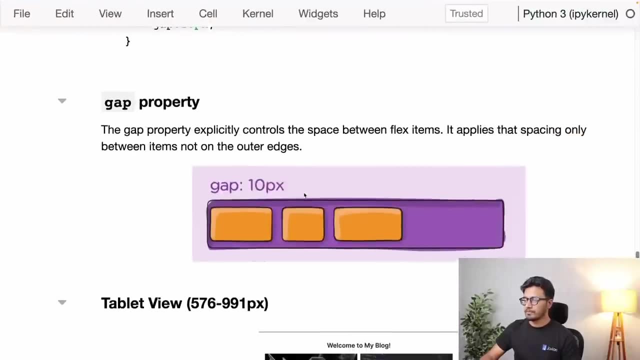 So there are a few various ways to add spacing between the card. The most efficient way that is used in the flex layout and that is the gap. So let's quickly see what gap is. So grab property explicitly controls the space only between the flex items. 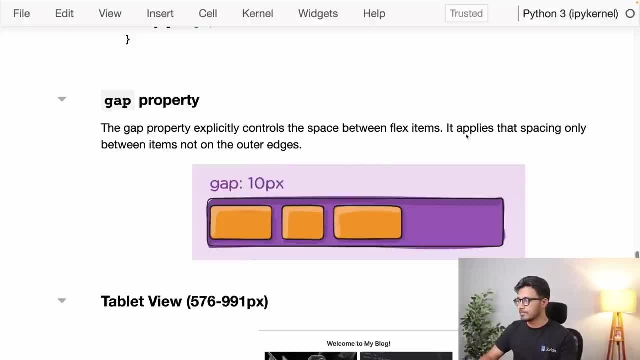 That are the children of a display flex layout. It applies that spacing between the items and not on the outrages. So the another way to do this is the margin top. But if you apply margin top, it will also apply to the first element, and we don't want. 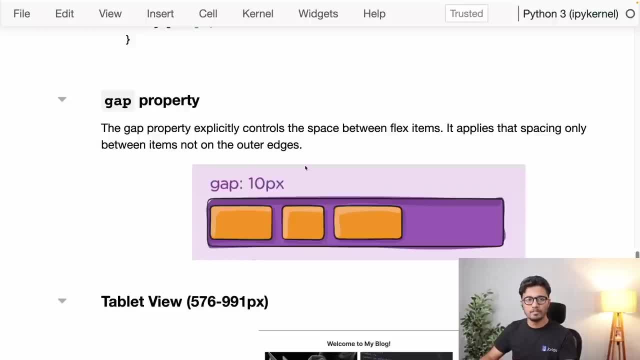 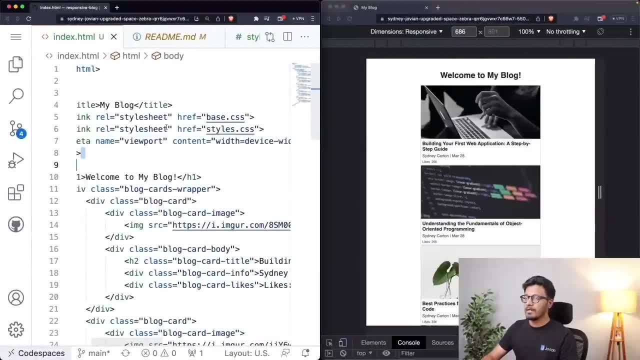 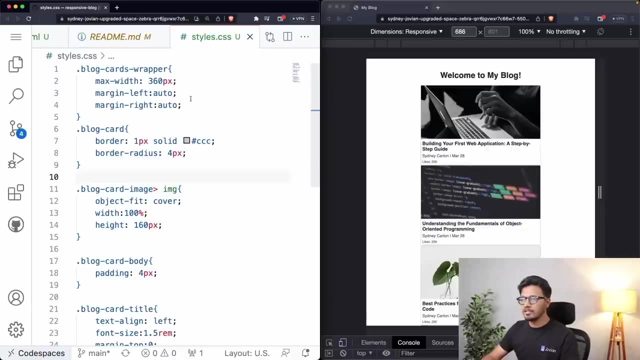 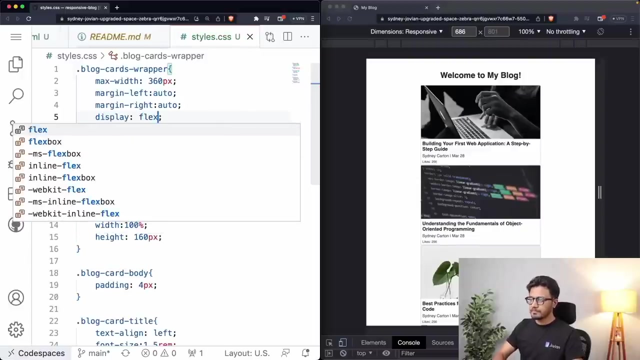 that We only want the spacing between the consecutive elements, So that's why it's best practice to use the gap, And gap will require us to. So currently we are not using any display property for this wrapper, So let's add a display flex property. 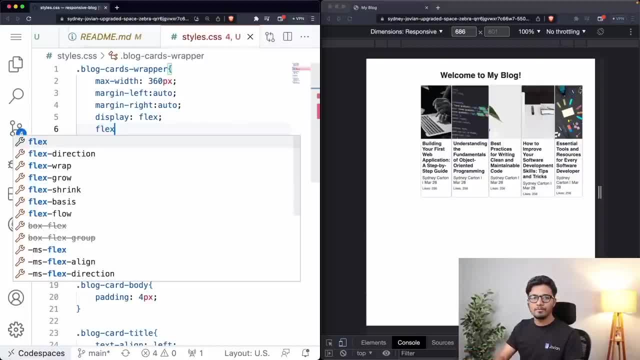 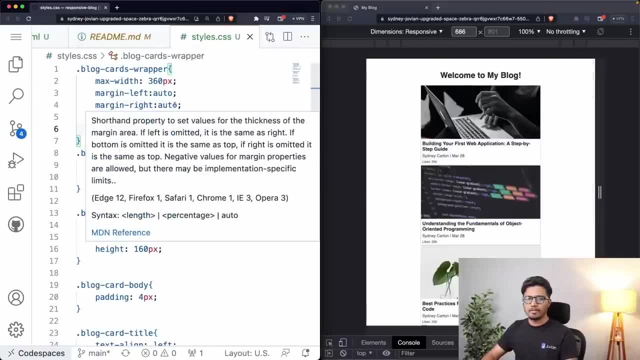 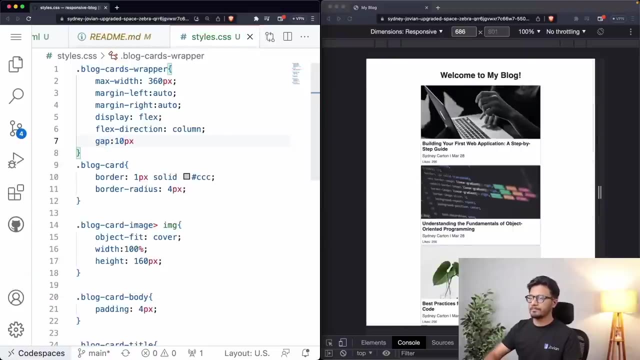 And the layout is in column format, So we will have to use flex direction column. Okay And Yeah, So we are now using the space property, which will be N P X. So now you can see that our mobile view is looking nice. 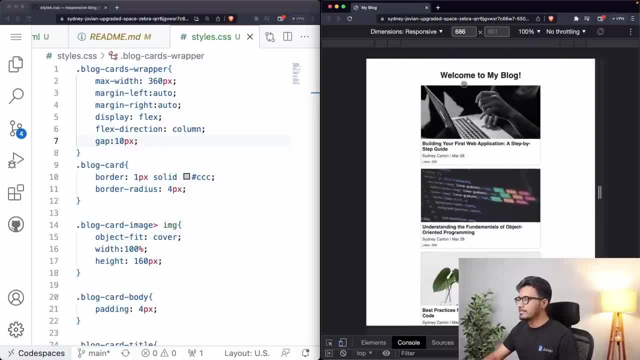 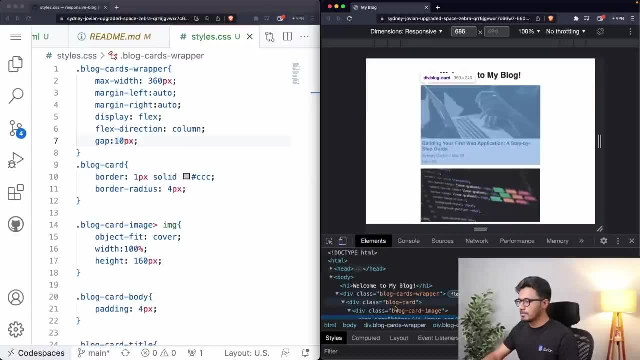 It is evenly spaced and there is no additional spacing here. that is applied to the card. So if we inspect this and we can see that there is no additional spacing applied here And the The, So the margin is highlighted using a color and there is no highlight of the margin here. so that is the. 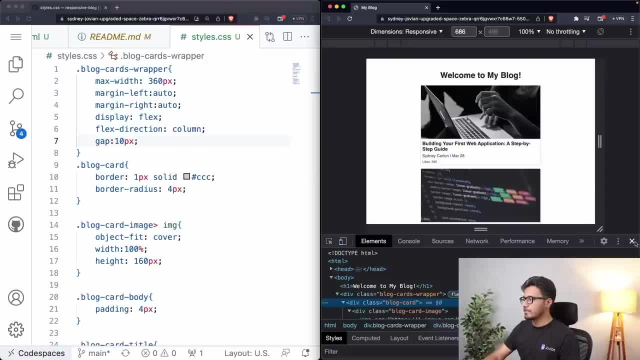 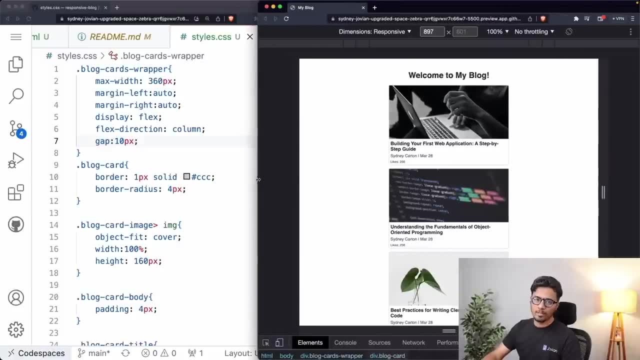 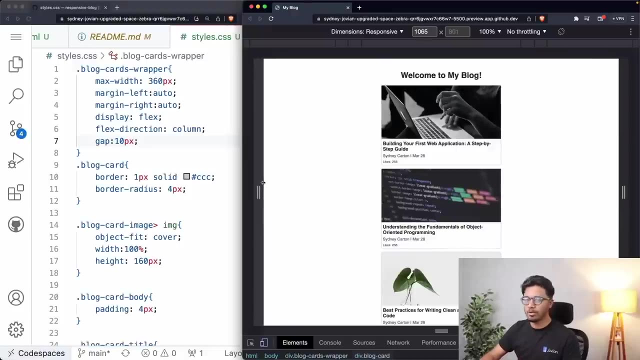 advantage of using gap. so we have uh completed our mobile view, so we so this is the mobile first approach, and we haven't written any additional rules that how our web page should look like on tablet and desktop devices, so it will look uh as it is, as it is looking on the mobile to make it. 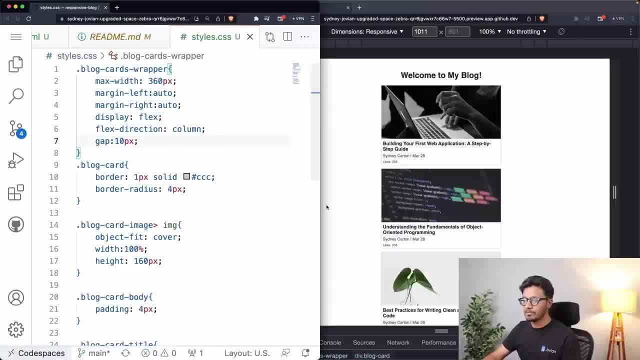 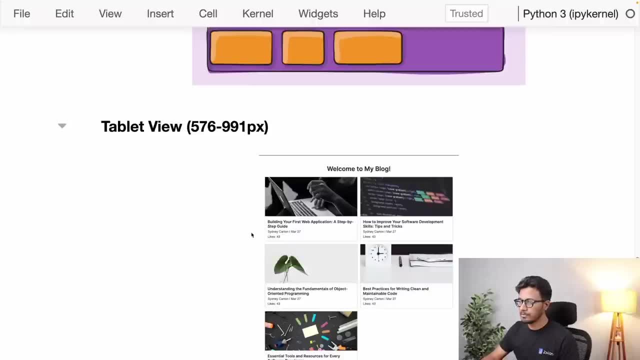 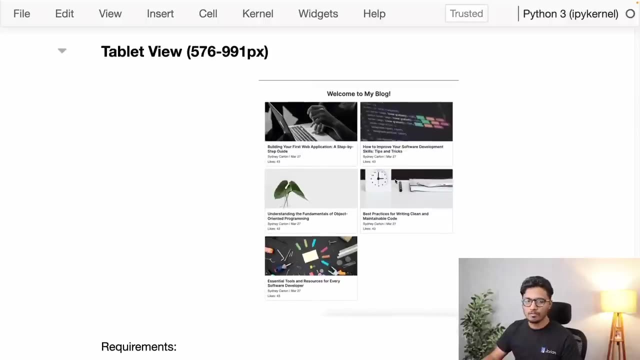 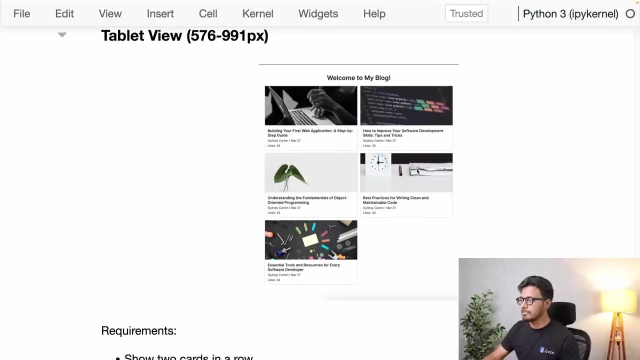 responsive to the other devices. we will have to use media queries with the breakpoints. so let's first design the tablet view. so in tablet view we want two cards in a row. so in this case we won't be using flex direction column, we will have to change it to row and also we will need some wrapping. 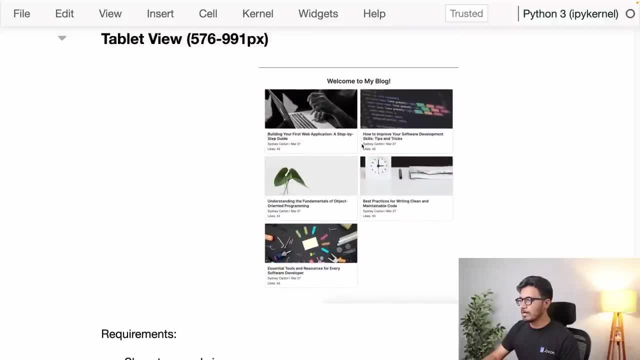 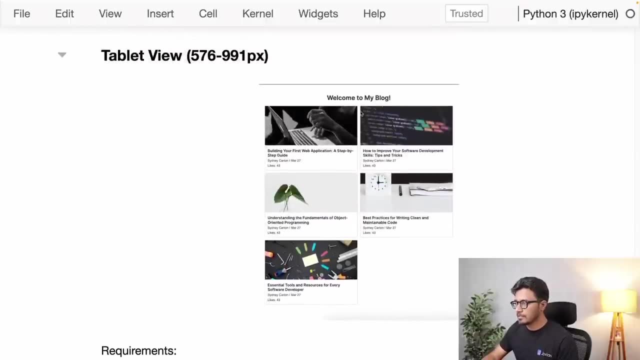 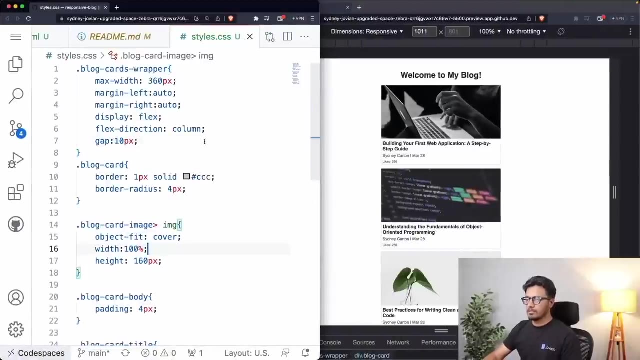 okay, so these are the requirements, and the spacing between the two cards, horizontally and vertically, should be 10 px, and all the cards should take the space exactly half of the available size. so for that we will need to add a media query. so let's add that. 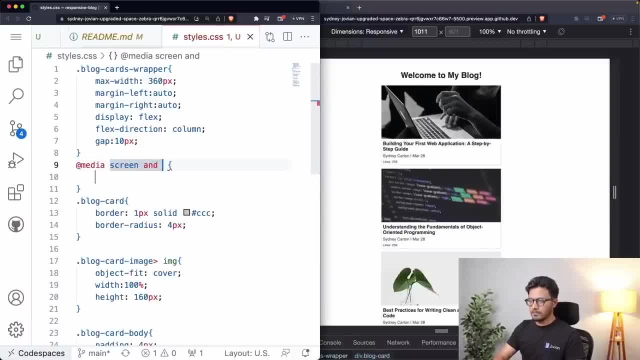 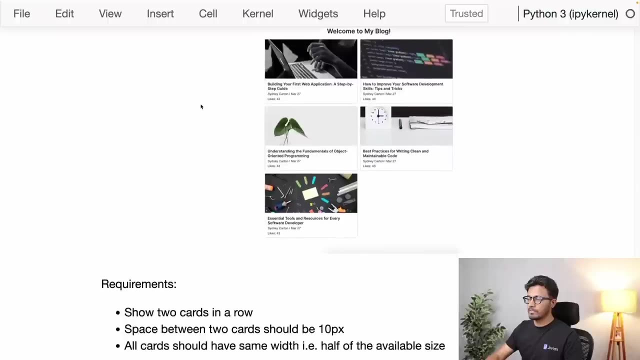 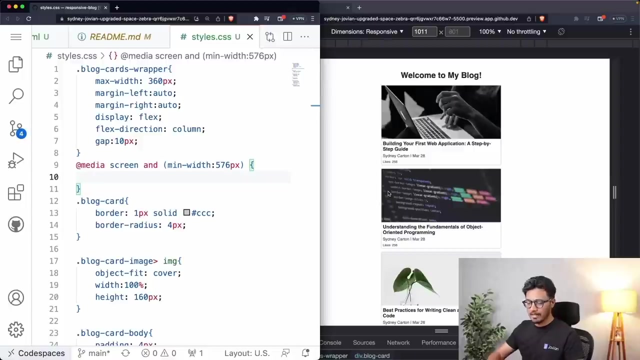 so we will require main width of 576 px. right. that is the breakpoint of the tablet and we first we will add the flex direction. that will be 15 px, and the following way: we will add the map of the tablet. we will add the map of the tablet. 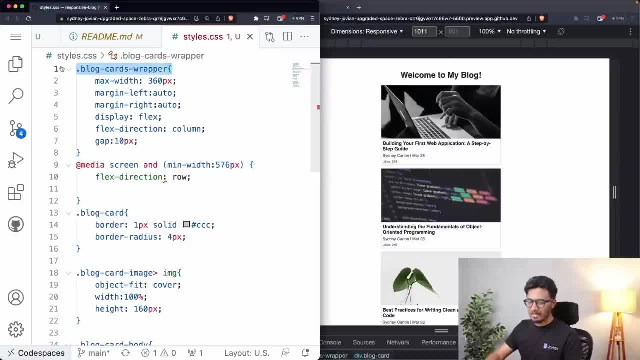 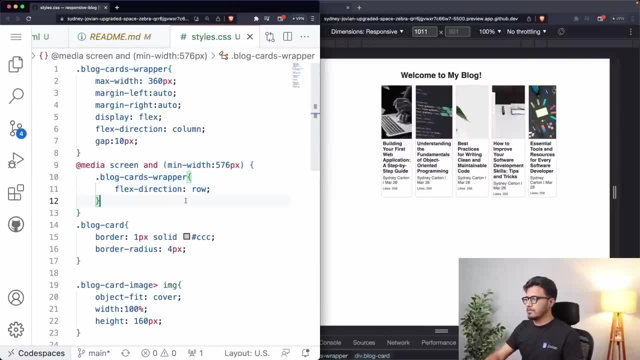 and also also we will add the class name of the tablet. so we will also need to add the class name of the tablet. so we will also need to add the class name here, so we can see that all the cards are coming in a single row. so to evenly space them and not to shrink them, we will have to use the property flex wrap. 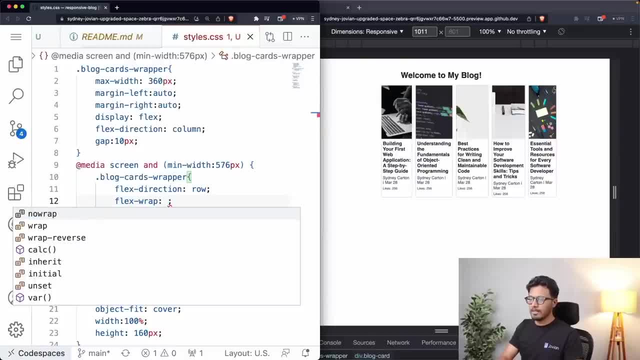 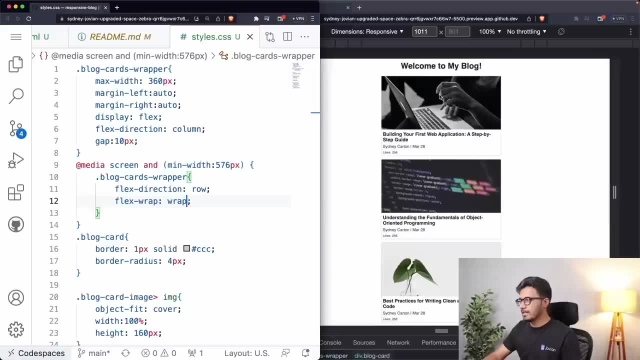 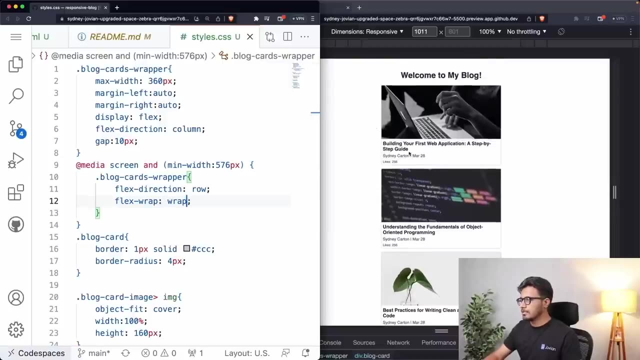 so we will add some extra space here and set it to wrap. so, after adding this, now you can see that all the cards are taking the space so that they fit their content correctly, but we can see that now if we are on the, let's say, tablet device we want. 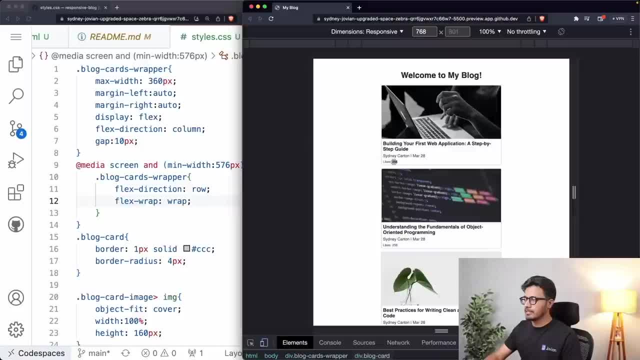 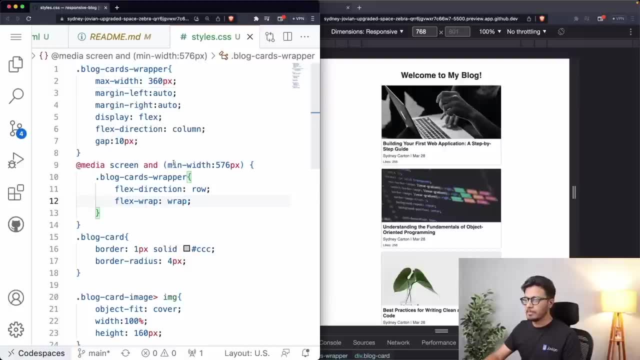 two cards in a row and it is just taking a single card in a row. that is because of the max width, which is set to 360.. so we will also need to modify the max width because now, for the tablet devices, we have more space available on our device, so let's update the max width to 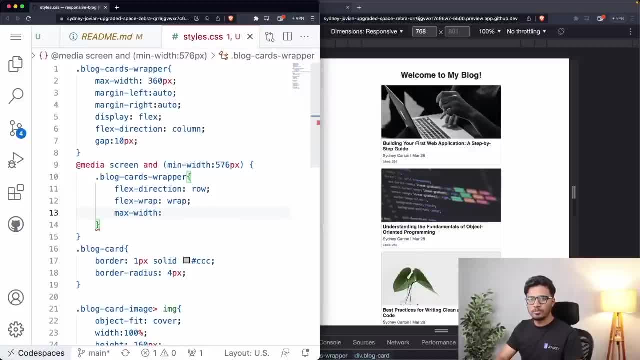 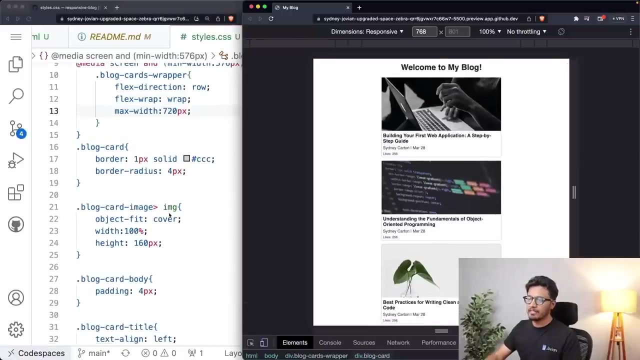 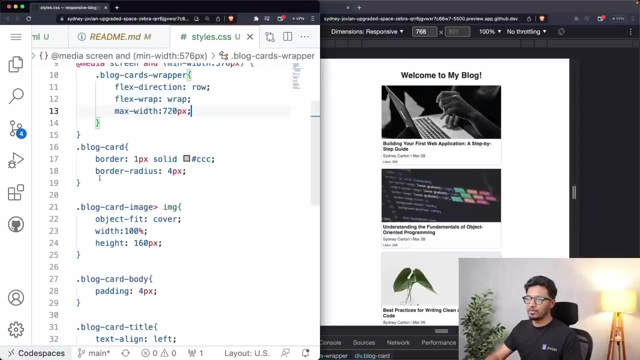 maybe we can double that, because now it should be less than 991 px, which is the boundary of the tablet device. so let's make it 720px, okay, and so still it will not work because we haven't specified any width to the block card and block card is still taking the complete width. so we'll have to add a property to the block. 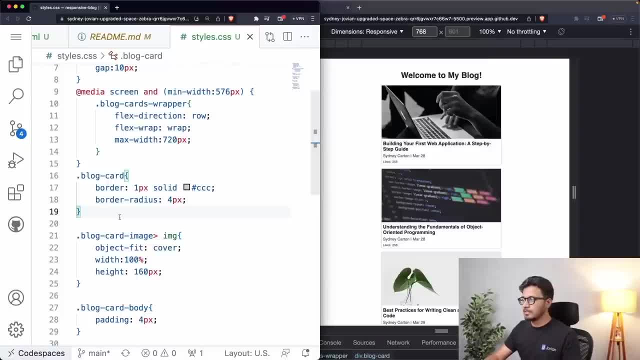 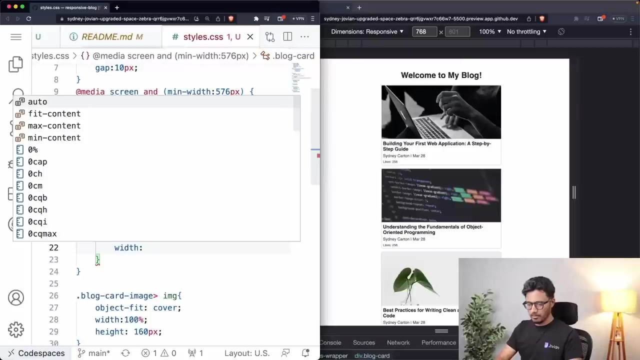 card to uh, to let the blocker know how much width it should take so that it can fit to in a row. so we can add this property again using the media query and we can put the block card class inside this media query and let's add a width of, let's say, 50 percent. 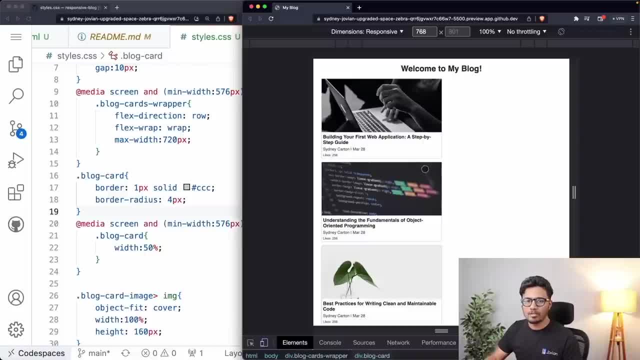 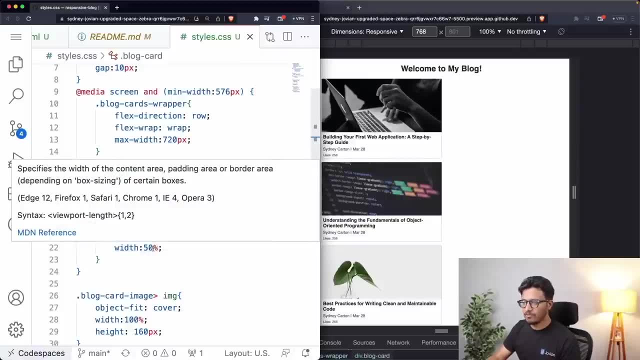 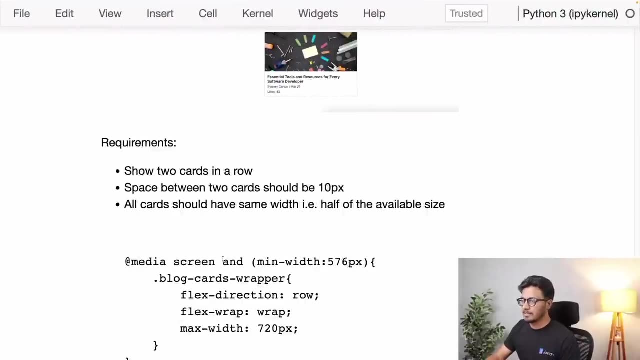 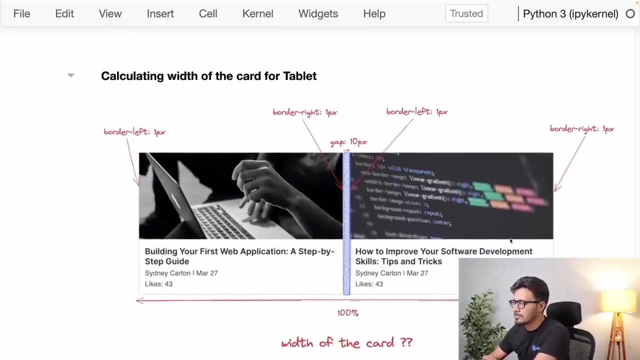 okay, so we can see that. still, it is not showing two in a row. so the reason behind this is we will have to check if 50 percent of the available width is available for the card or not. so let's understand the concept here. so we want two cards in a row and there is already a gap of 10 px between the two cards. 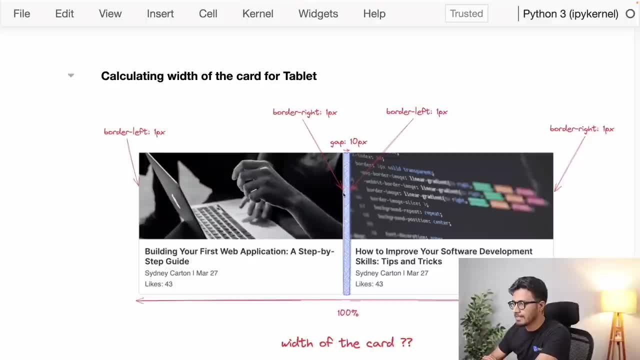 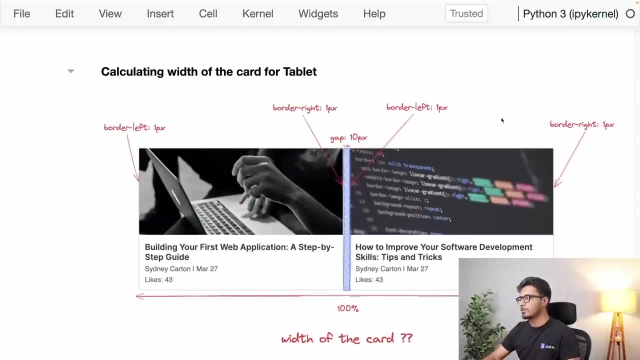 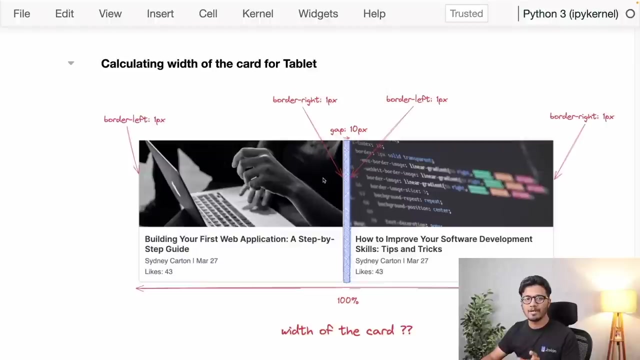 and each card has a border on the left and the right side and the border width is 1 px. so in total 10 px is gone from 100 percent and uh compute like so in total for the border is taking 4 px. so the actual available width is 100 percent minus 10 px for the gap and 4 px for the border. 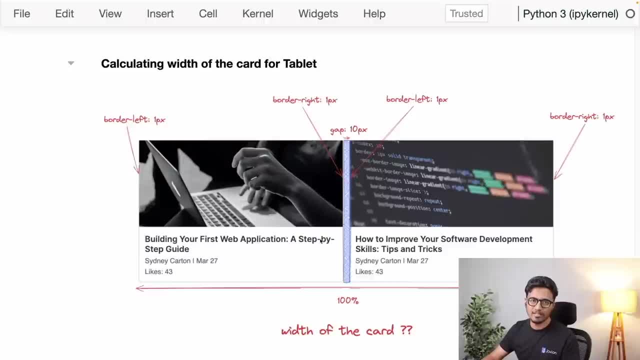 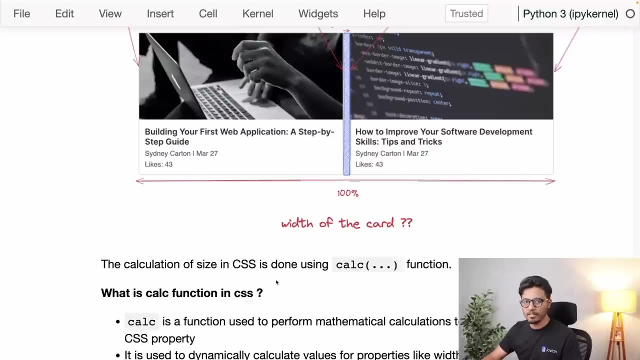 so that much width is available and that needs to be divided into 2, and if we give that, then only the cards will show two in a row. so how to do this? so in css there is a way to calculate the width or any other property, and that is done by using the. 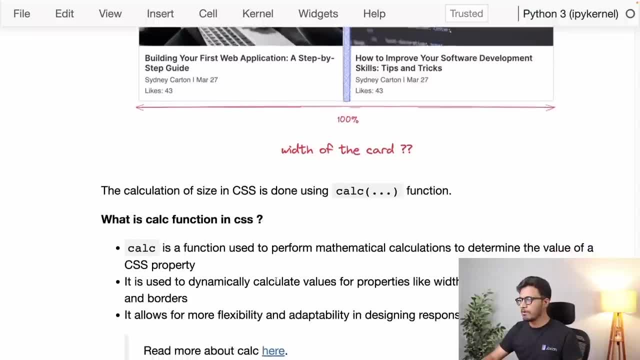 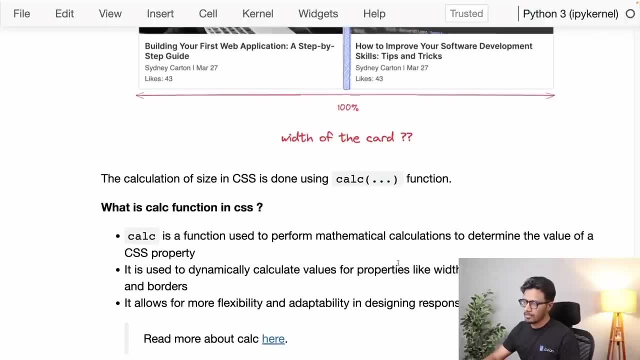 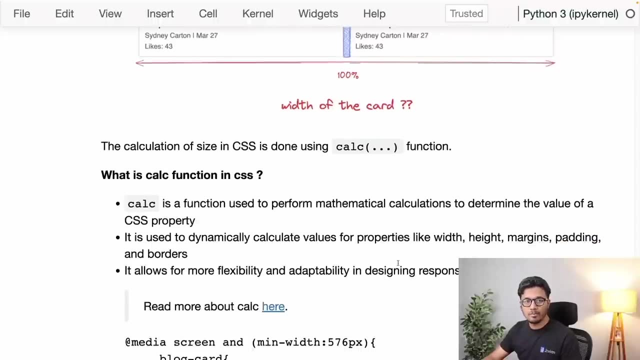 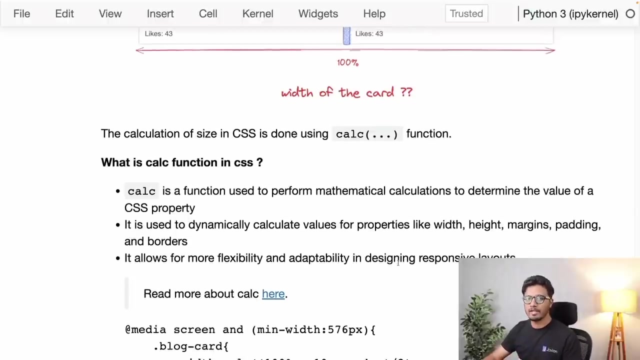 calc function. so calc function is used to perform mathematical calculations to determine the value of a particular css property. so it is used to calculate the values dynamically and it is allows us to make more flexible layouts and even if we resize the screen, it will automatically recalculate the values. 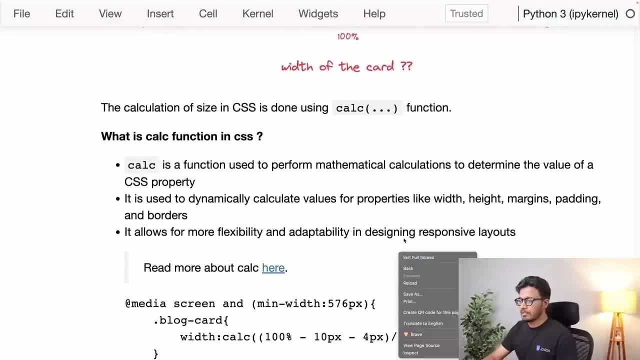 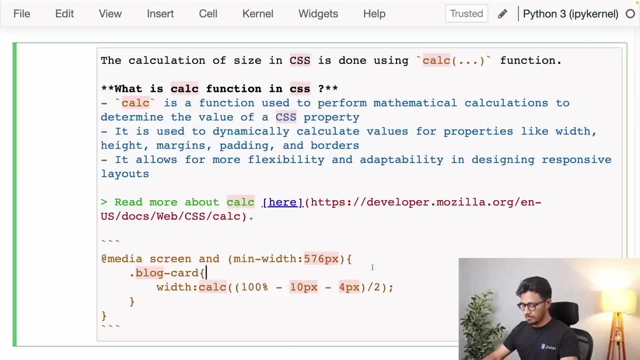 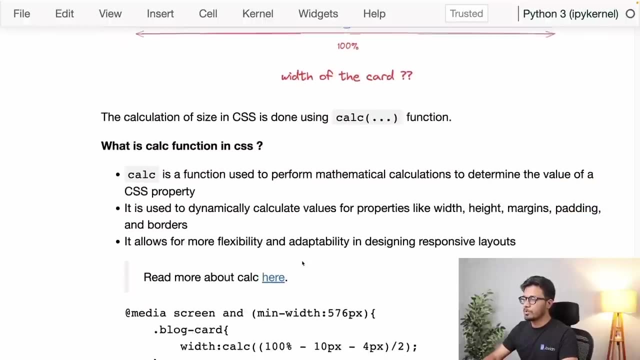 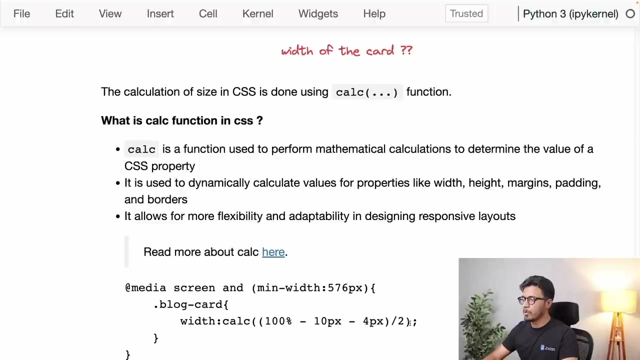 and apply it to the elements. so to do that we will have to use the width property and the calc function. so inside the calc function we will put the calculation that we want to do so out of 100 percent. 10 px is for gap and 4 px is for border, and the remaining width we will divide into two parts. 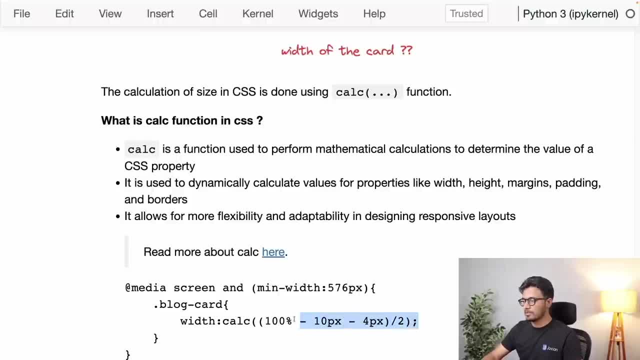 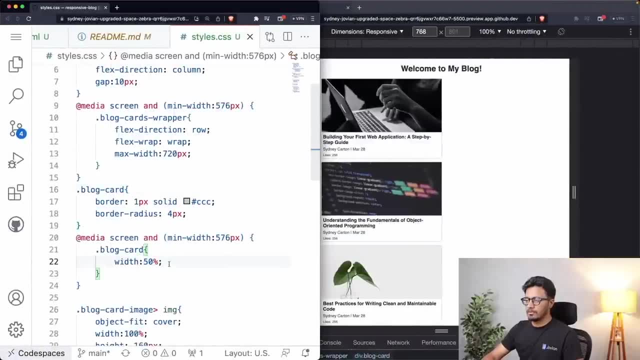 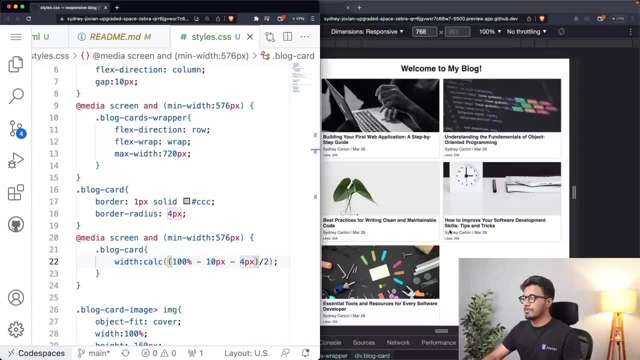 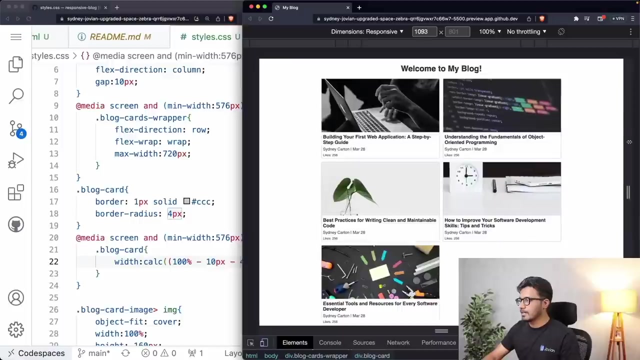 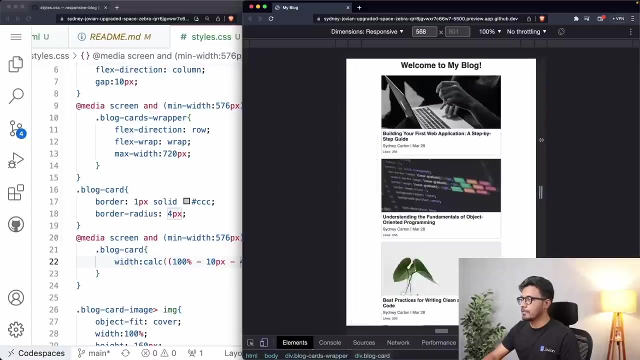 two, because we want to show two cards in a row. so let me add this width to this block card. inside this media query, just make the plot of that cell to the 小 with the value of 1, so we can see that the block page is looking correctly on the tablet device. 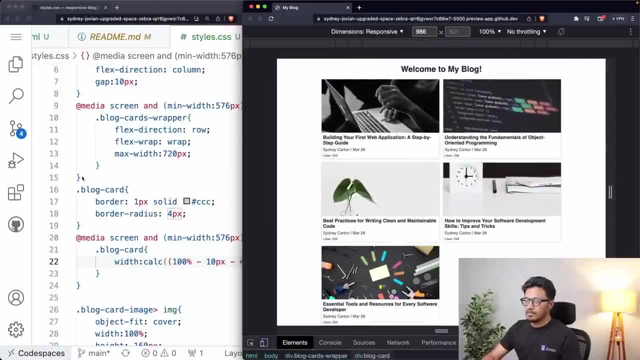 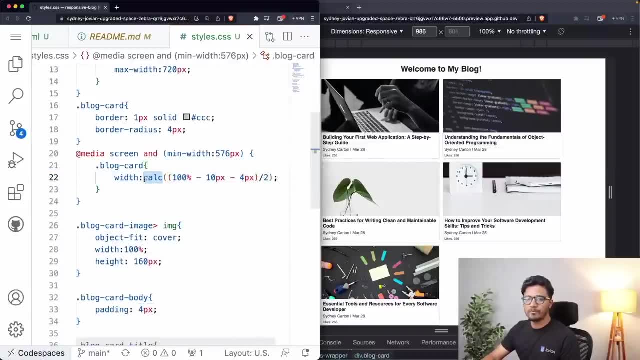 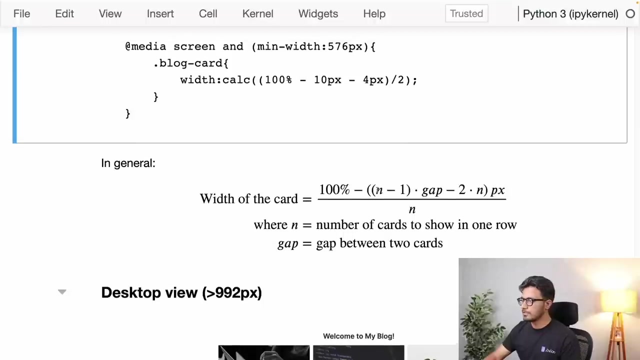 and from 576 it should change to tablet view, and below that it is still taking the column layout that is expected from the mockup. one line of code: here we were able to make our web page responsive for tablet. now similar thing we will have to do for desktop, so for desktop. so this is the formula that we can use in general. 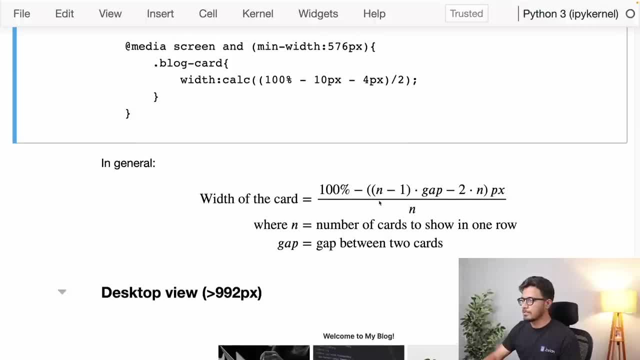 to calculate the width of the card. so here, 100 percent is the total space in width available and n minus 1, where n is the number of cards we want to show in a row and gap- gap is 10px in our case- minus 2 into n. so n is again the number of cards and 2 represents the border on the left and 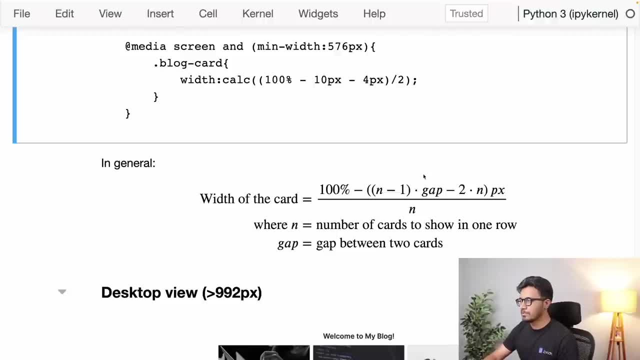 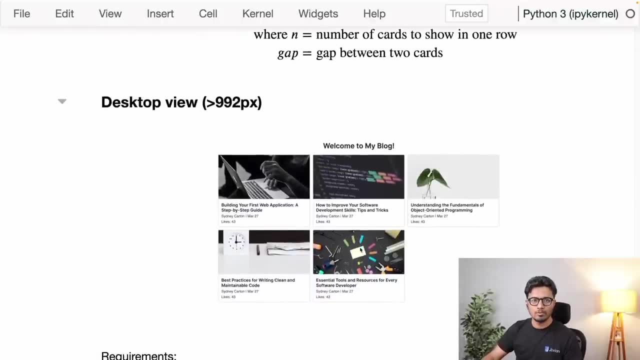 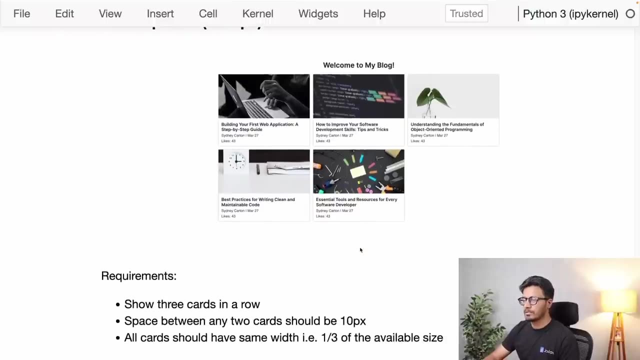 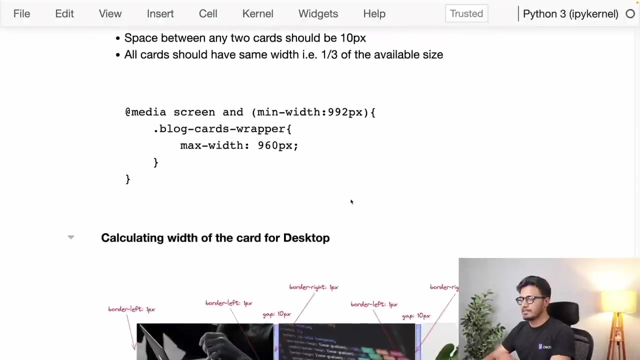 the right side. so if we put 2 in this formula we will get the same expression. so for desktop view we want to show three cards in a row. so for showing the three cards we will have to again calculate the width by substituting: n is equal to 3, so let's understand again how it is done. so this is the hundred percent width, which. 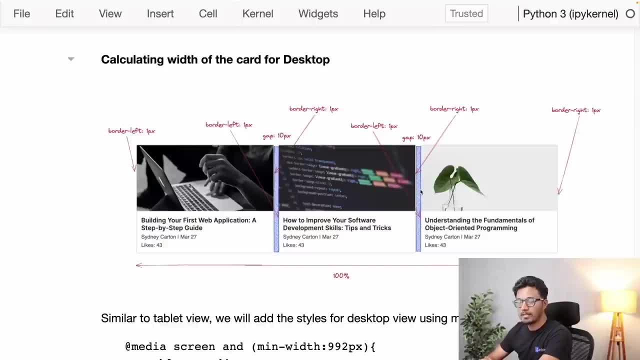 is available. out of that, there are two gaps because we have three cards in a row, so there will be two gaps, 10px each. so in total the gap is taking 20px space and border left and border right: 2px per card. so in total we will have: 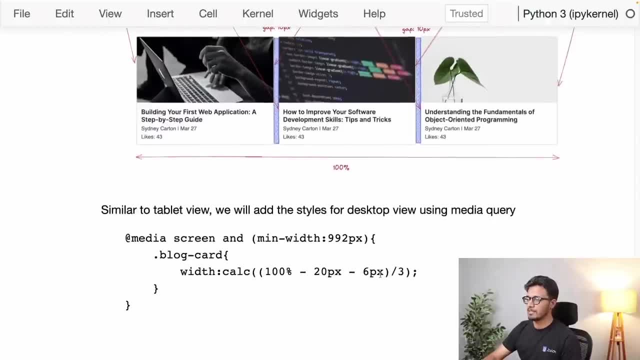 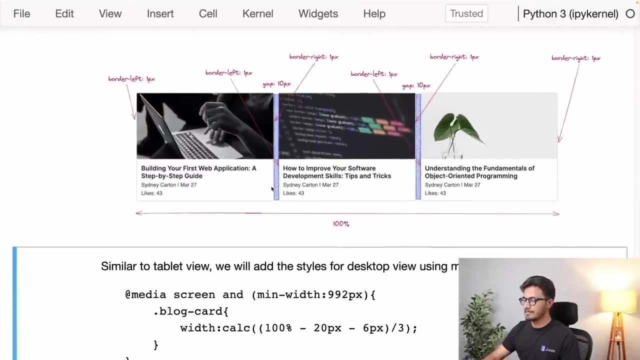 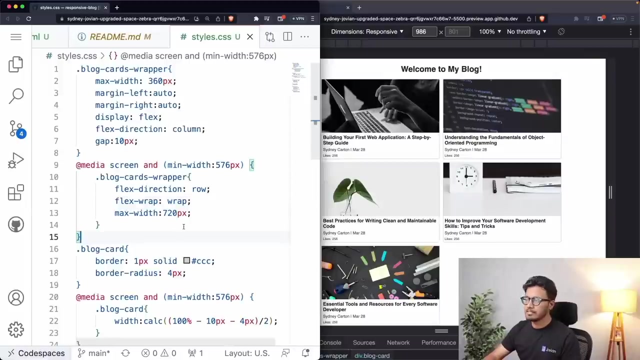 to subtract 20px and 6px and then divide the remaining space into three parts. so this is how the block page will become responsive for desktop. let's try to quickly add this. so, uh, for desktop, now we have larger screen width, so we can change this 720px to maybe. 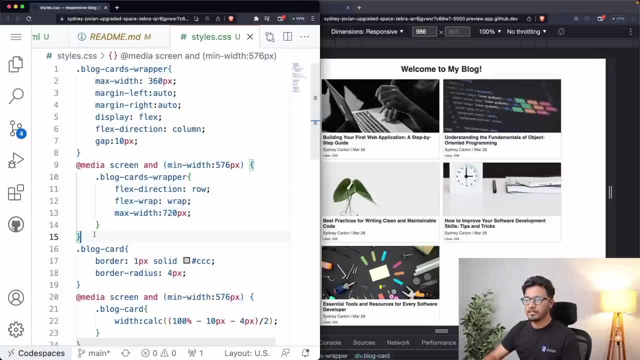 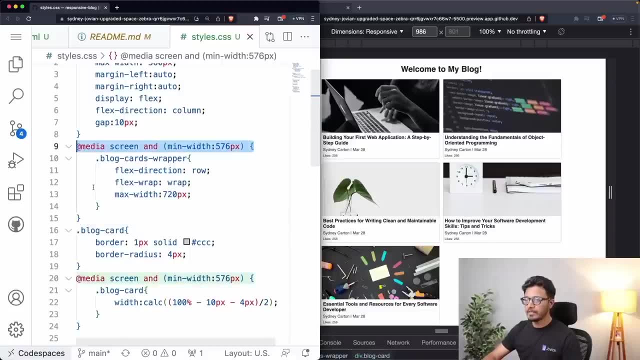 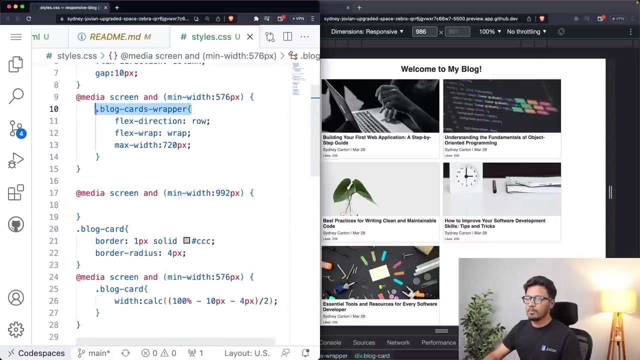 some more device, because now we have space uh till 991px. so I will copy this media query and change the minimum width to 991px, which is the starting- sorry, 992px, which is the starting point for the uh desktop devices, and put the blocks card starter. 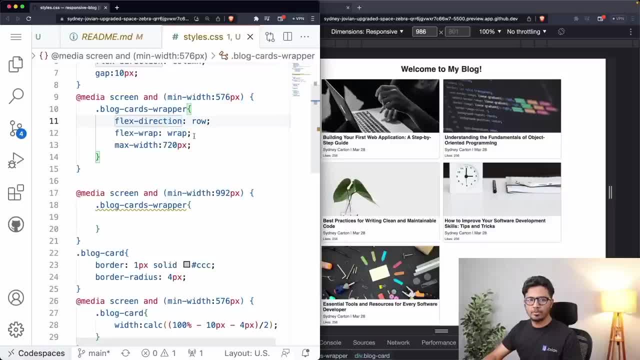 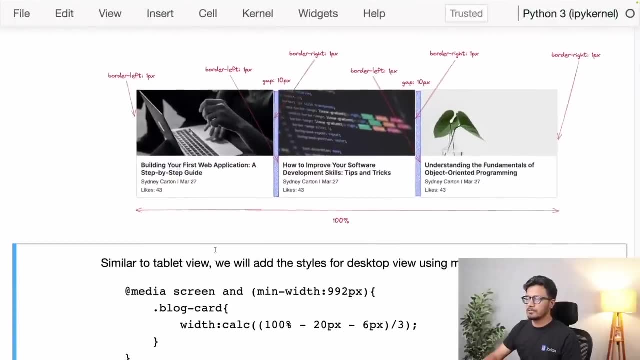 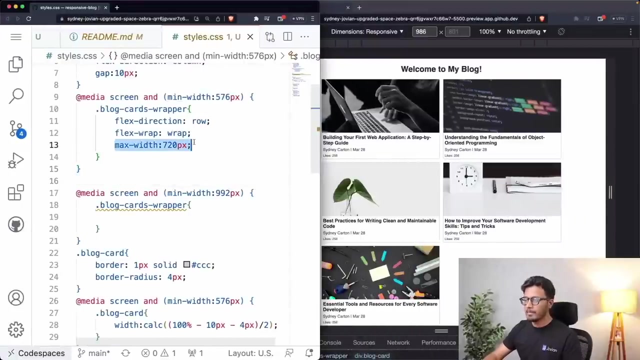 and we can see that these two properties. we don't need to again copy that because, uh, on the desktop view itself we will be requiring the row flex direction and we want them to wrap. the only property that we need to change is the max width, because we now want three cards in a row. so let's copy only the max width and add that here. 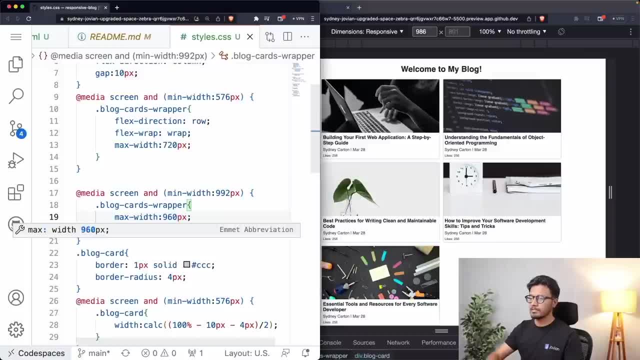 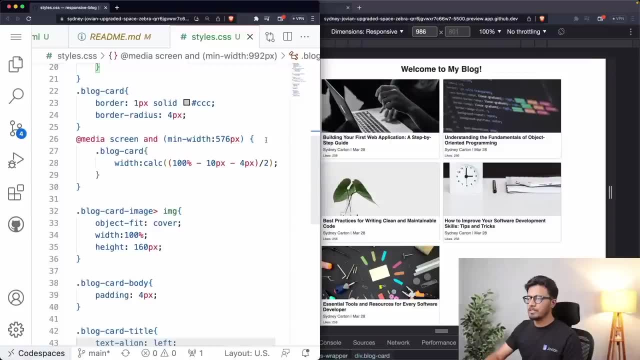 and let's say we make it 960px and similar thing, we will have to add a media query for the block card. so here the minimum width will be 992px and the width will be 20 hundred percent minus 20px and the width will be 20px. 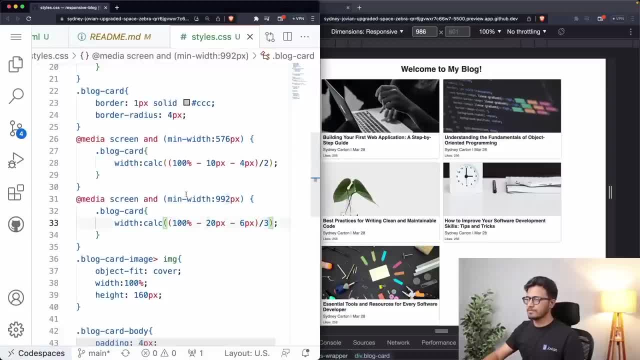 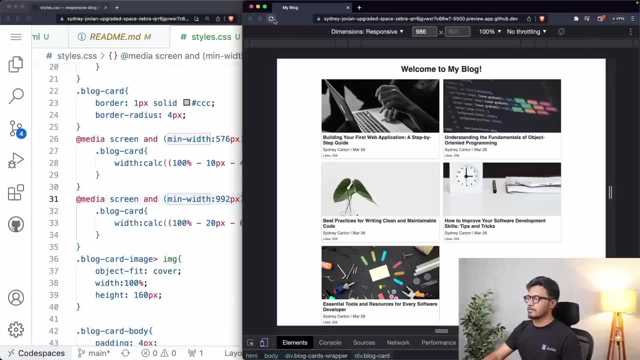 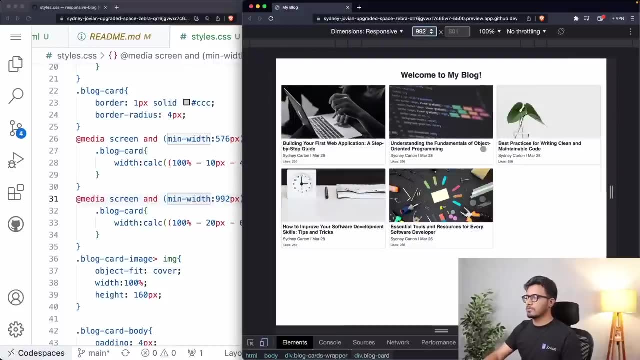 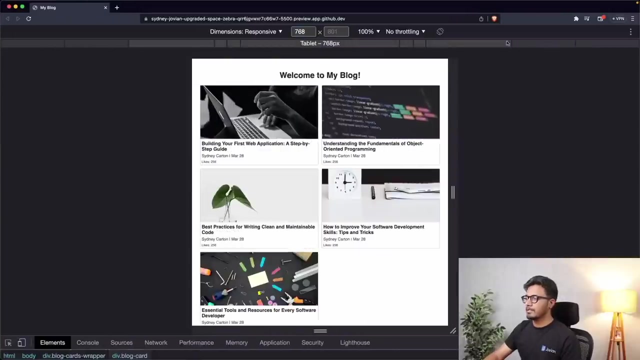 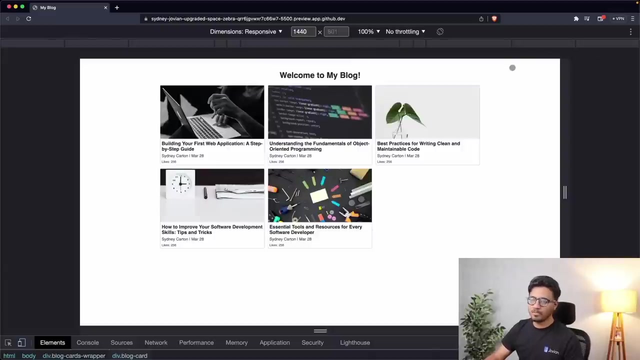 minus 6px divided by three. so if we go to 992px, we can see that now three cards are shown in a row. so this has made our web page fully responsive for mobile, tablet and desktop and, if you want to make it more responsive by making use of the screen width of the higher devices. 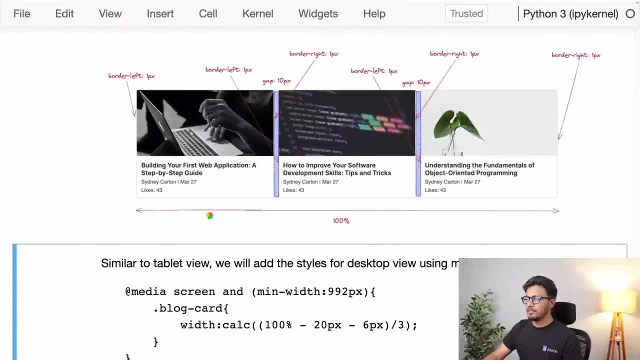 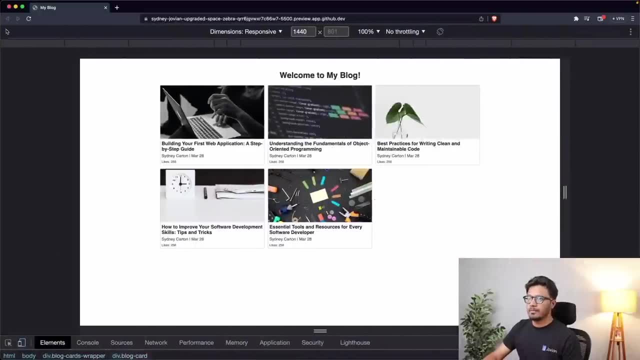 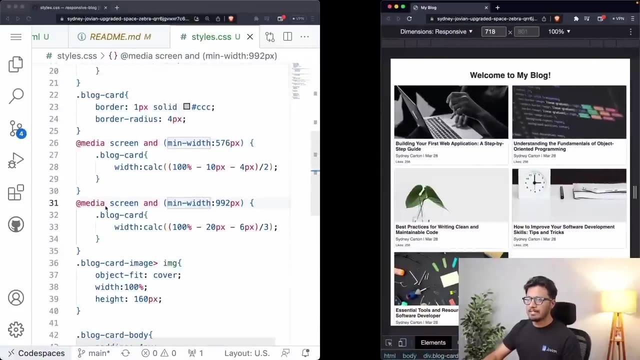 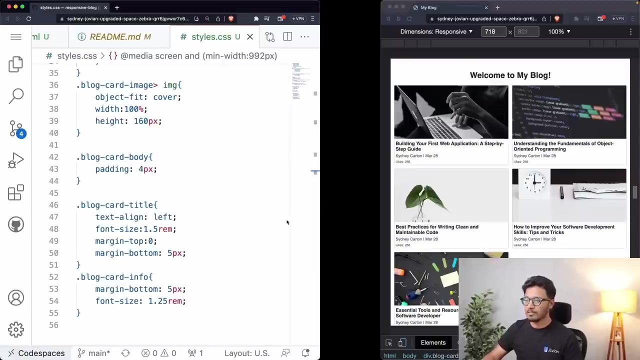 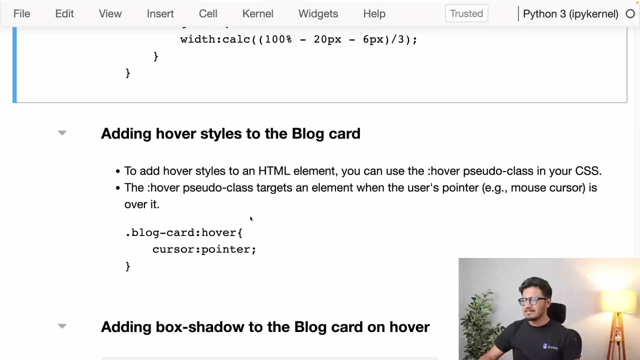 you can add the screen, you can add more media queries and can make that more responsive for the higher devices. so you can see that we have added less than 60 lines of code css and have created a responsive block page design. so now let's understand some other properties of css. 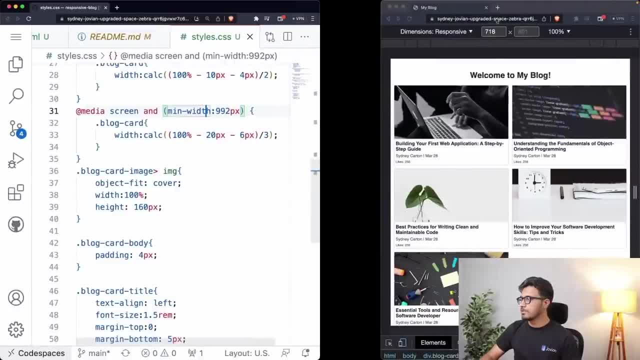 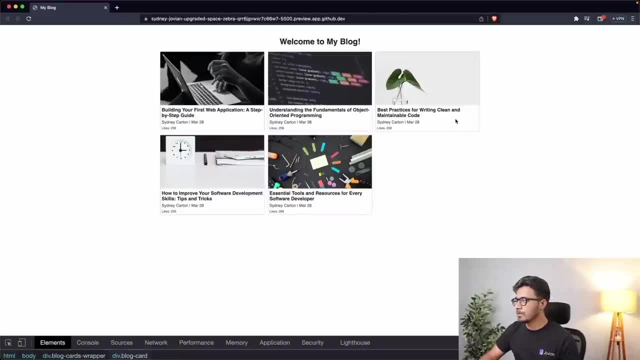 for adding the whole styles. so suppose we want to add some whole styles to the card. so right now if we hover using the mouse over this card it is not changing the style. but let's say we want to add some shadow to the card and also want to change the cursor of this card. 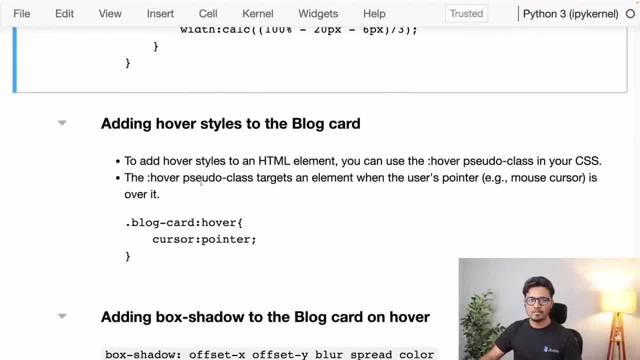 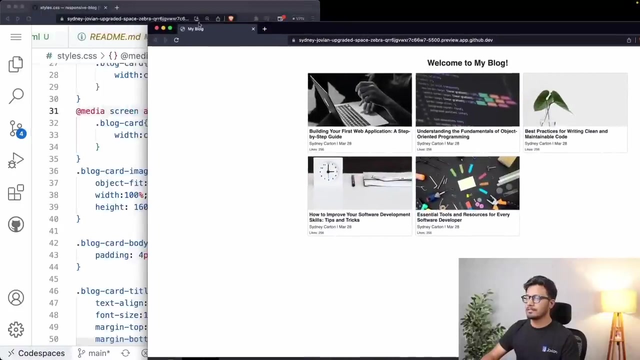 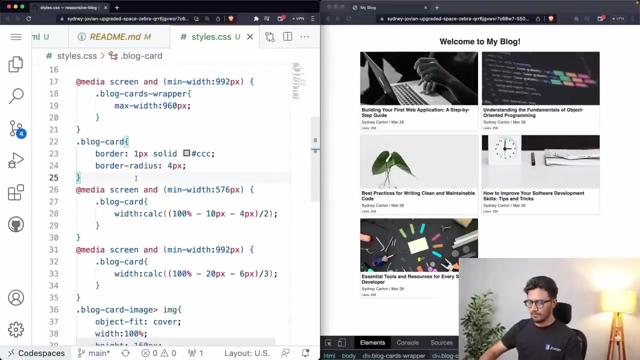 so how can we do that? so for that css provides some pseudo classes. so the one example of pseudo class is the whore. so to add styles to the pseudo class we have to use the selector colon and name for the block card. we will be using the whole pseudo glass and let's try to add that. 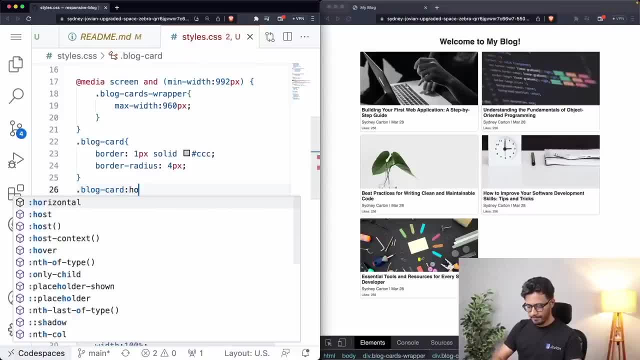 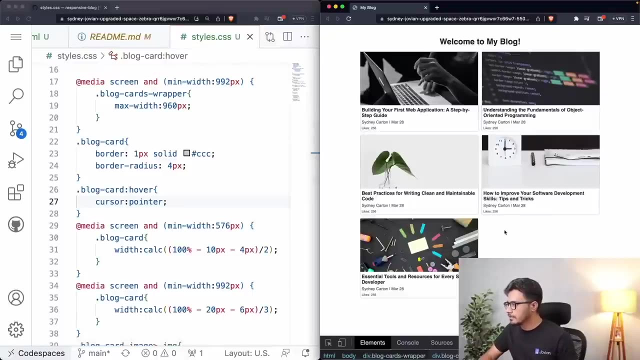 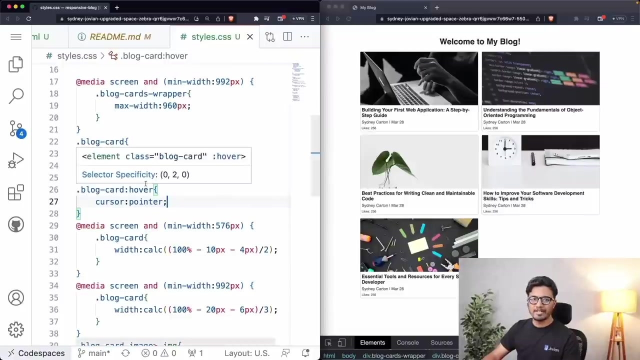 we can add it here and add cursor pointer. now you can see that the default pointer device is the arrow and when i hover any card it is showing me the pointer device. so in the similar way we want to add some shadow to the card to indicate that the mouse is over that particular card. so for doing that we have a box shadow. 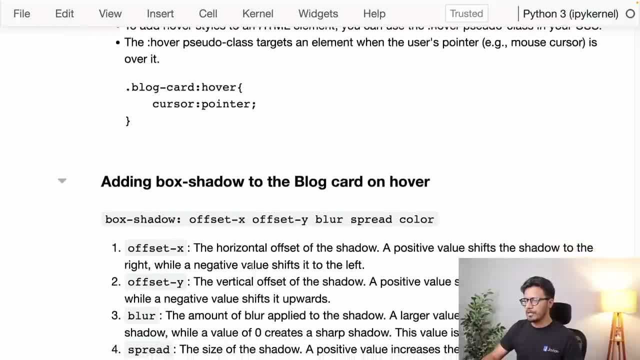 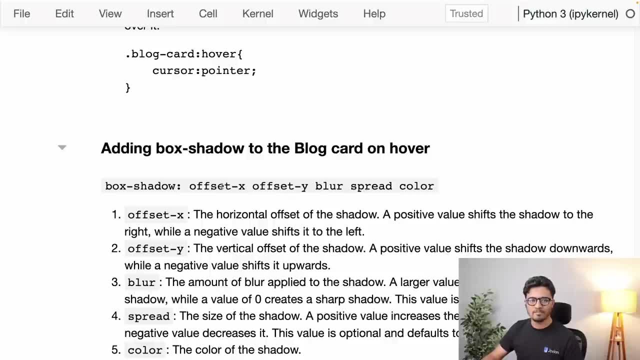 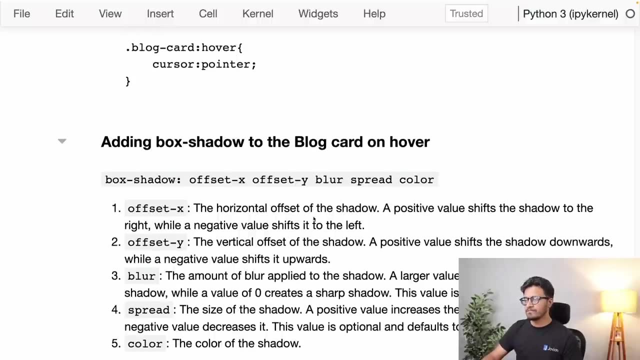 property in css. so the way of specifying the box shadow is in this way. so it accepts five parameters: first is the offset x, second is offset y, third is the blur spread and last is the color. so offset x means how you want to position your shadow. if you specify some positive value here. 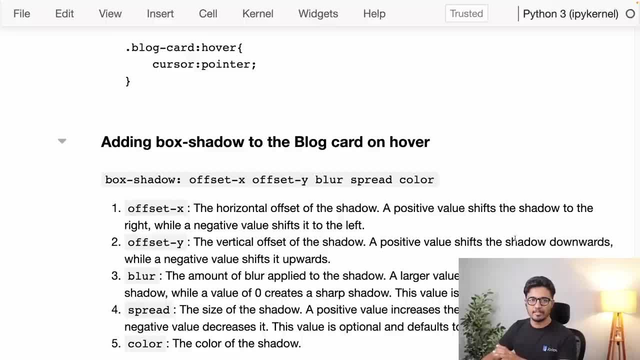 the shadow will shift to the right side, and if you specify negative value, it will shift to the left. same thing applies for offset y. if you specify positive value, it is going to shift downwards, and if you specify negative value, it is going to shift upwards. there are few more. 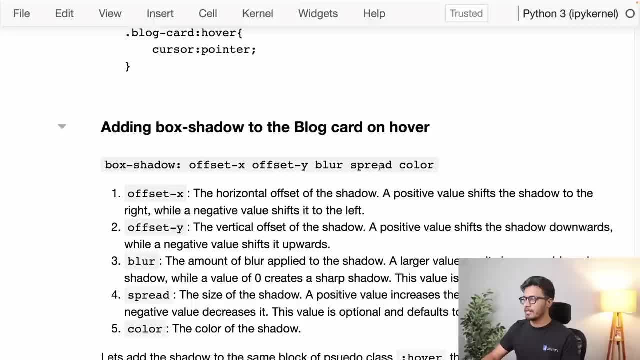 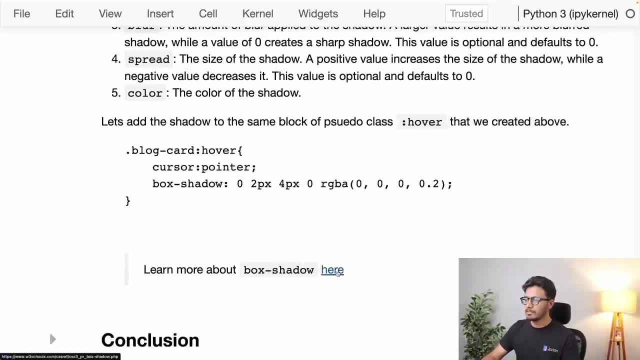 properties that you can use to position your shadow. so, for example, if you specify positive properties of the shadow, one is blur, spread and the color of the shadow. so you can check this out. i have provided a link here which specifies some more properties and how specifying these. 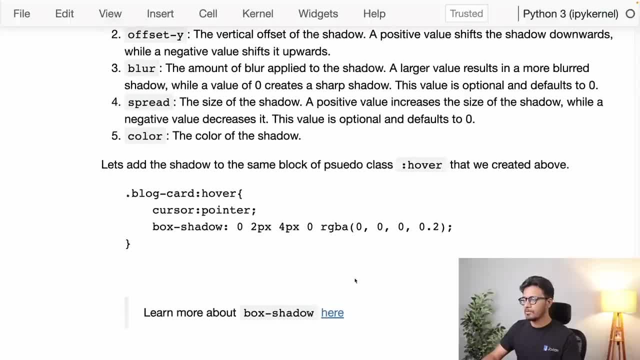 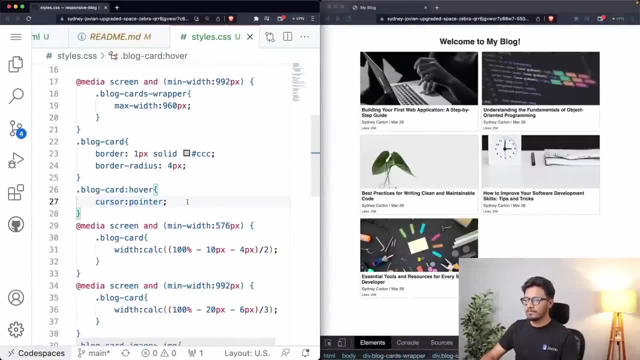 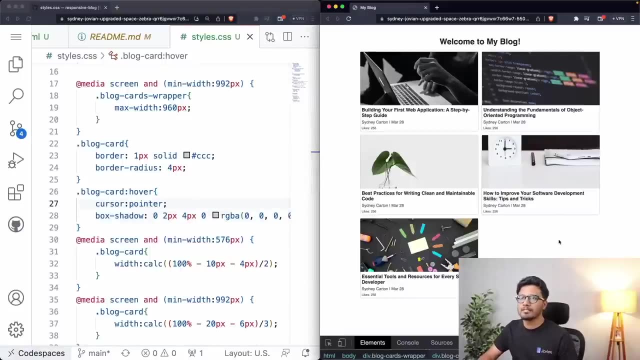 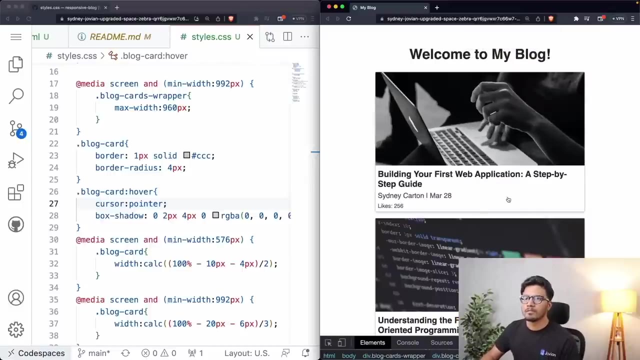 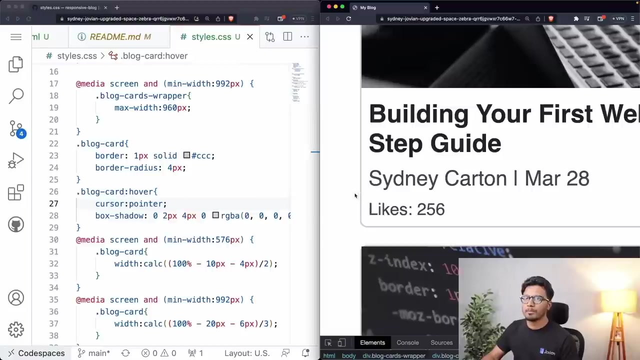 different values how the shadow changes, so you can play around with that. for now, we will use this shadow property and add it into the for style so you can see that. let me zoom in a bit so you can see that there is a shadow here which appears when we hover over the card. 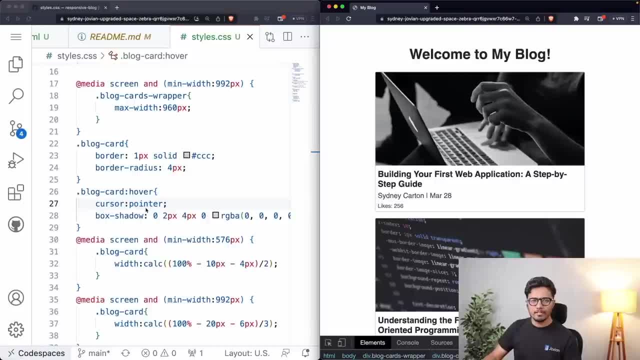 so in this way we can also change the background color of the card. if we want to hover, also we can change the color of the card if we want to change the color of the card, if we want to change the font size. all the colors and font size can be altered here if we want to do that on hover. 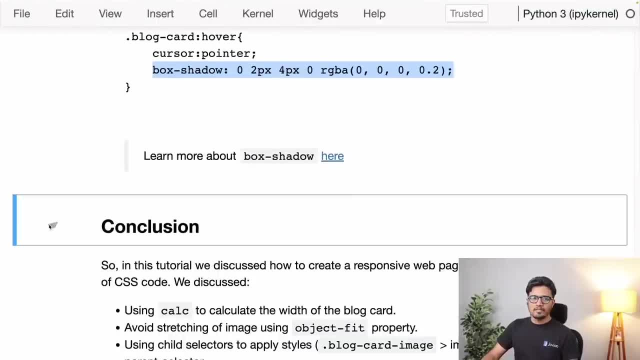 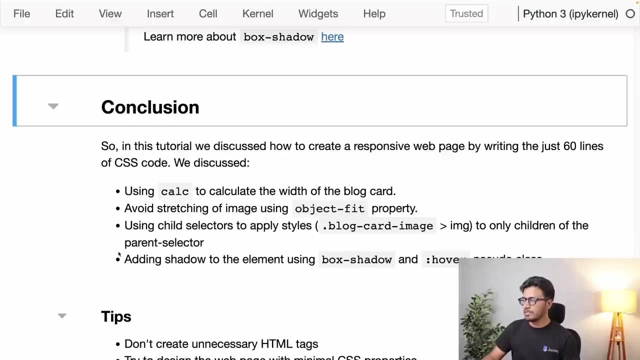 all right, so that's the end of the session. let's conclude. so in this tutorial, we learned how to create the responsive web page by just writing less than 60 lines of css code, and we learned how to use calc function in css to compute the width dynamically for our block card. and we also use the object fit property. 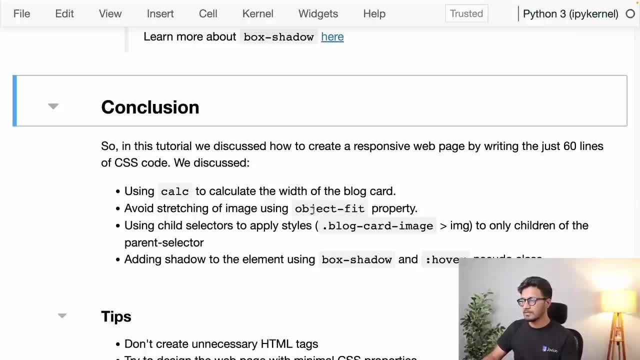 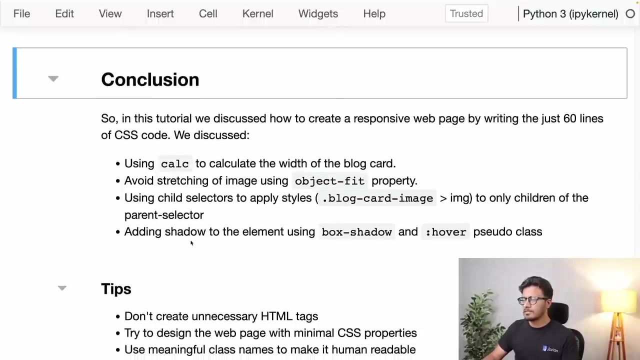 so that the block images are not stretched. we also learned the child selectors. if we want to apply styles to a particular element inside a particular selector, that can be done using child selector. there are few more child selector that you can check. i have provided the link and. 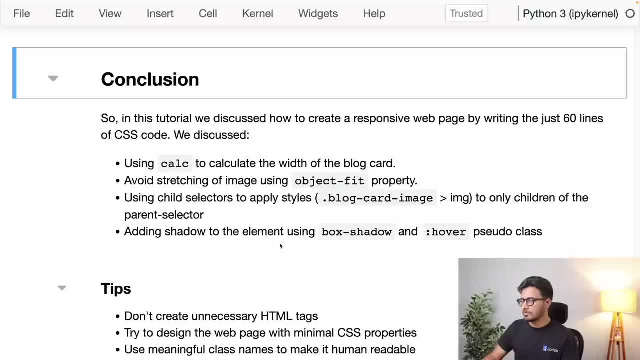 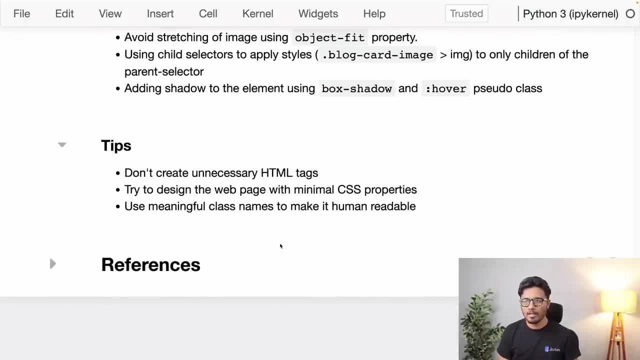 also, we learned how to add a shadow to the card using the sudo class her. a few tips that you should keep in mind. so don't create unnecessary html tags and try to design the web page with the minimum tags, and same thing applies for the css properties. don't add unnecessary. 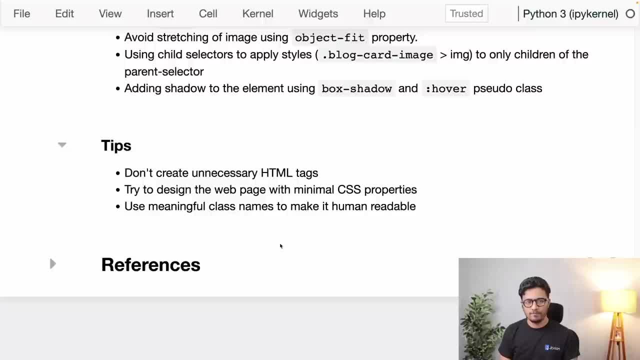 unnecessary tags. 1958 leap base. so don't create unnecessary text collections. don't create unnecessary, unnecessary CSS properties. Check if the display flex is whether really required or not. If it is required, then only add. Otherwise it will become very hard to scale on various 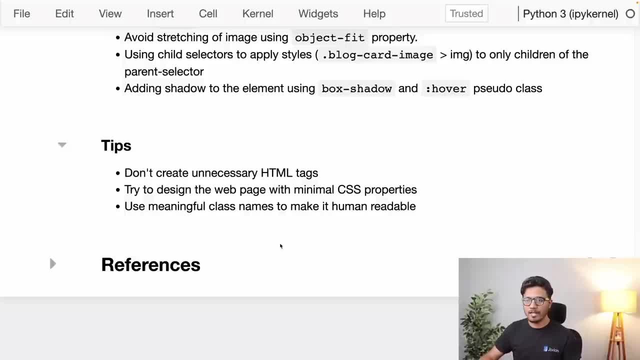 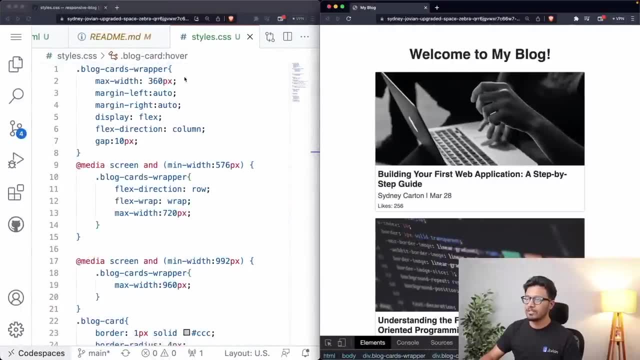 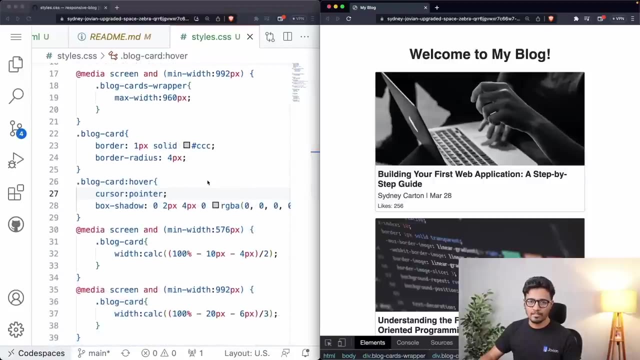 devices And, lastly, use meaningful class names to make it human readable and signify what they are doing. So if you look to the class names that we have used, so all have a meaning to what element they are representing on our HTML page. 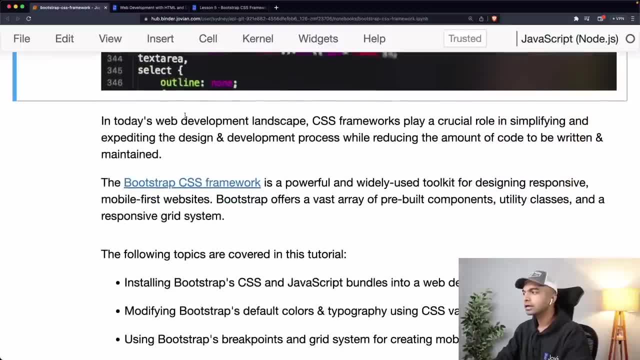 In today's web development landscape, CSS frameworks play a crucial role in simplifying and expediting the design and development process. You've been building web pages for some time now And you may have seen that a lot of effort goes into making sure that. 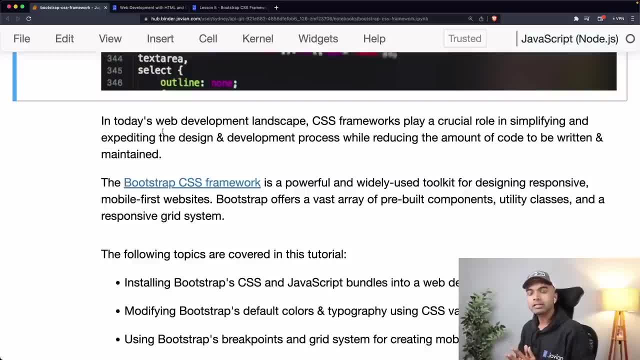 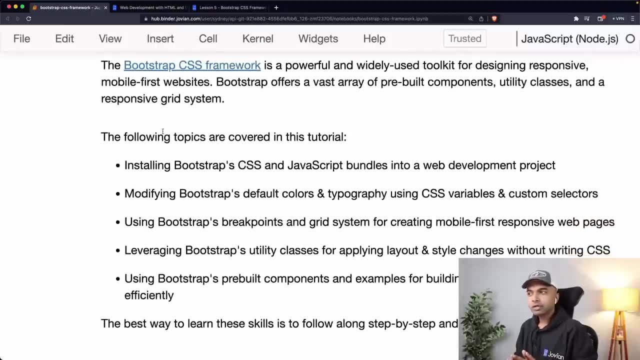 things look. things look exactly how you need them to, And this is where CSS frameworks can help Reduce the amount of code that needs to be written and make the process of web development more efficient. We're going to talk about the bootstrap CSS framework today, which is: 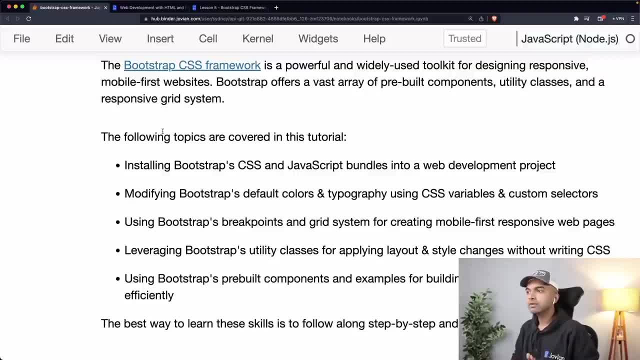 a powerful and widely used toolkit for designing responsive and mobile first websites And bootstrap. bootstrap offers a vast array of pre built components, utility classes and a responsive grid system, which also makes it very easy for you to work with Flexbox without actually having to write a lot of flex properties. So today we're going to see. 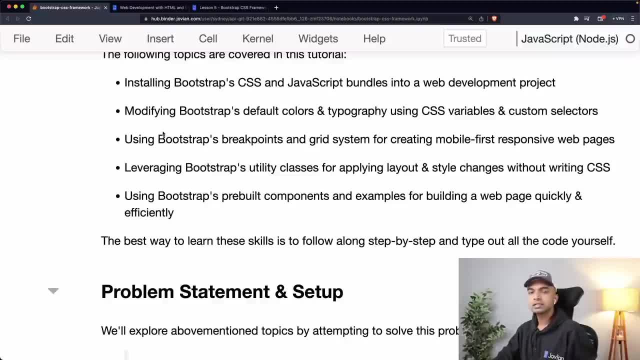 how to install bootstraps, CSS and JavaScript bundles into a web development project. we're going to learn how to modify bootstraps, default styles, which is, colors and typography, using CSS variables. We're also going to learn how to use bootstraps, breakpoints and grid system. 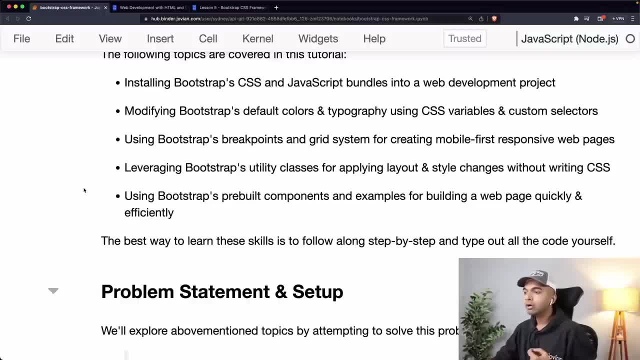 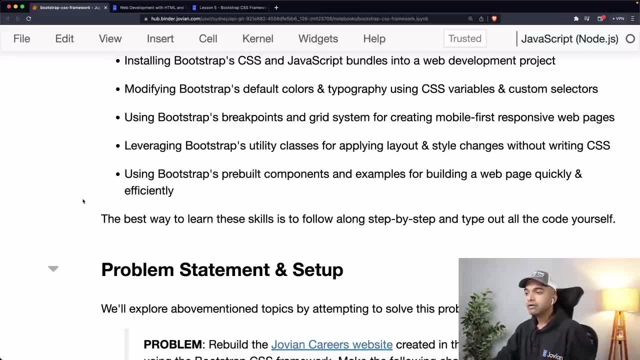 for creating mobile first, responsive web pages. We'll talk about leveraging bootstraps- utility classes for applying layout and style changes without writing a lot of CSS. And, finally, we'll also use bootstraps- pre-built components and examples for building a webpage quickly and efficiently. 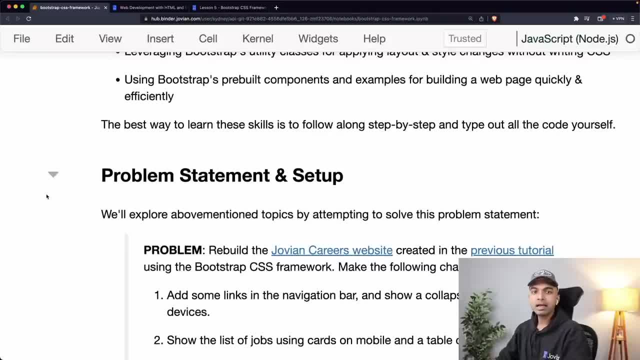 And the best way to learn these skills is to follow along step-by-step and type out all the code yourself. So I highly encourage you to do that. The more code you write and the more you ask yourself about every line of code you write. 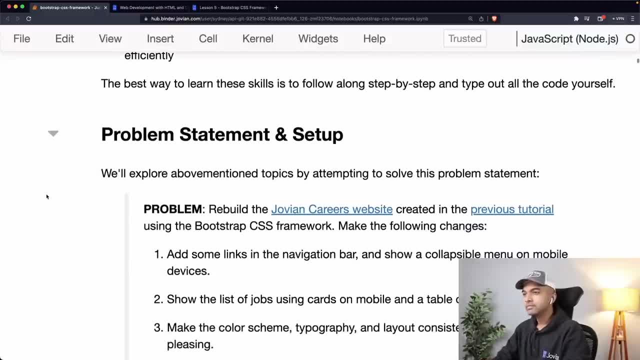 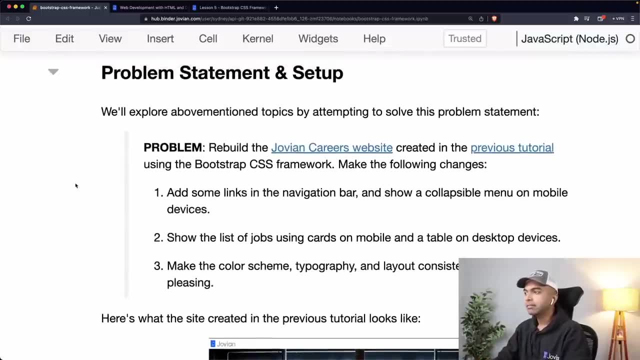 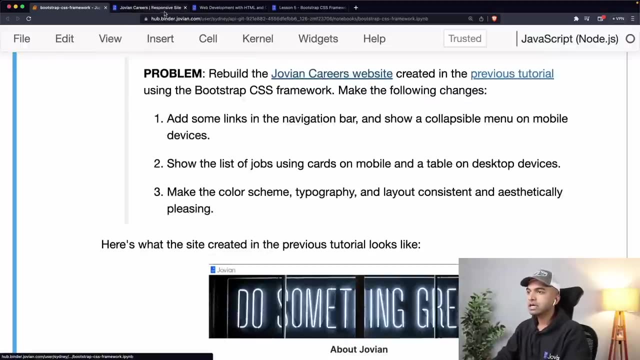 the better you will become as a web developer. So always make sure that you understand every line of code that you're writing. So we will explore these topics by attempting to solve this problem. statement. Over the course of the past few lessons, we have been building a Jovian careers website. 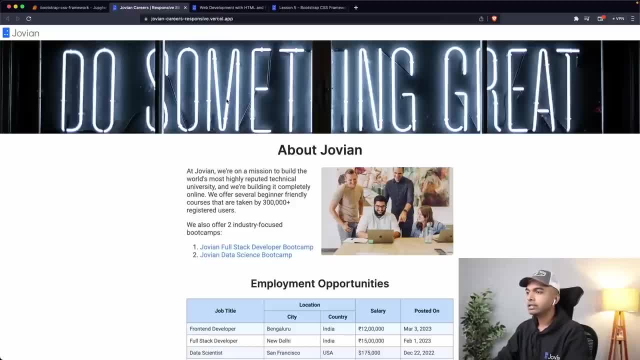 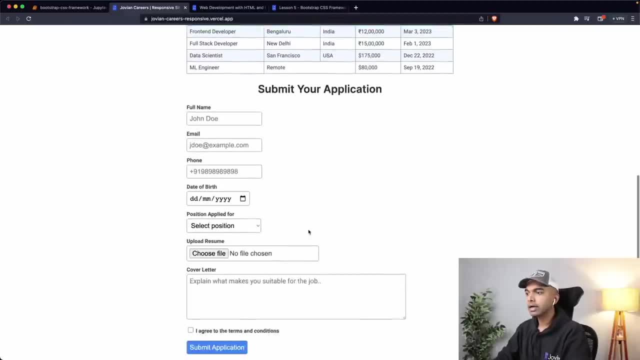 So here is what it looks like: There is a nav bar here at the top, then there is a banner image and there is an about Jovian section, followed by some employment opportunities, a table followed by an application form, followed by a footer at the bottom. 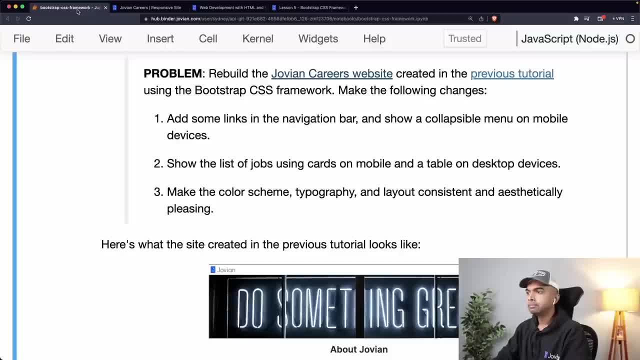 So this is the website that we have been building so far, And in today's lesson, in today's tutorial, we will rebuild this Jovian careers website using the bootstrap CSS framework. Now, the reason we are rebuilding the same site again and again is to understand how. 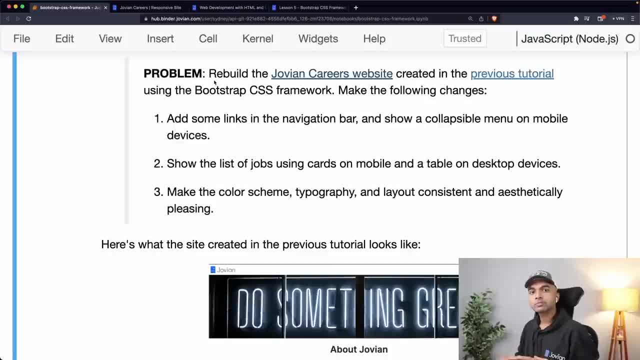 to make the web development process more efficient while at the same time, improve the aesthetics and the completeness or the finish of your websites. Okay, So I would like you to just keep that in mind today, that you will notice today that we are writing less code. 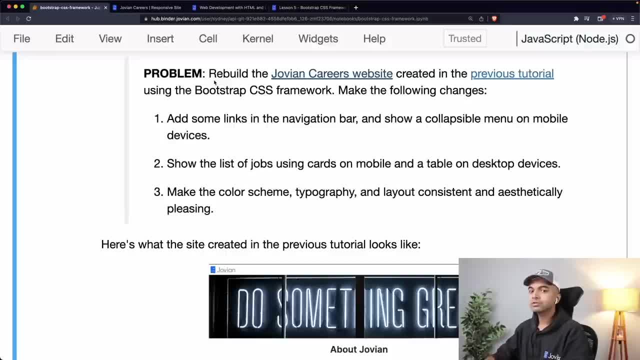 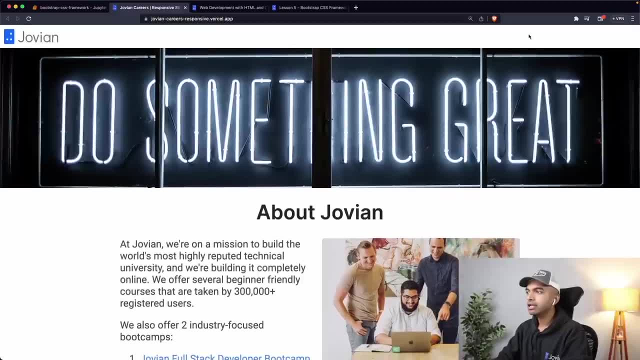 But we are ending up with a better website, And that is something that makes you far more efficient as a web developer. So, specifically, we will add some links in the navigation bar as well. So here we have a navigation bar. we'll add some links here at the top. 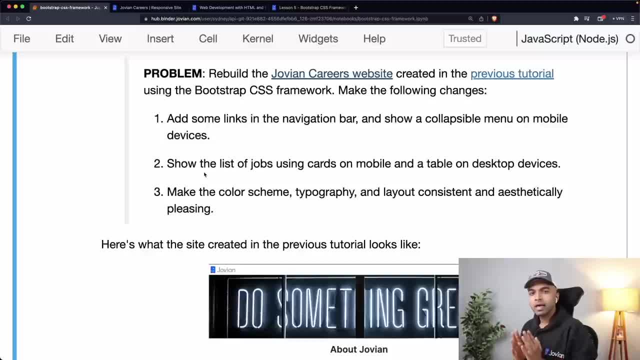 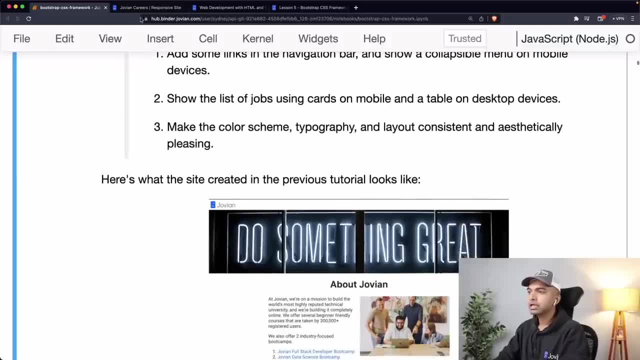 And we will also then make that collapsible on mobile, because you don't have a lot of space to show links on mobile, So we'll add a menu button over there. We will also show the list of jobs using cards on mobile and using a table on desktop. 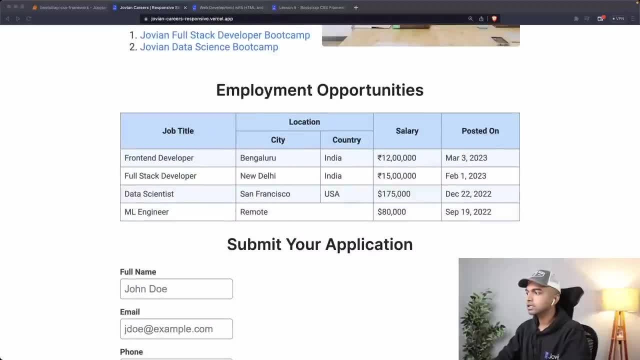 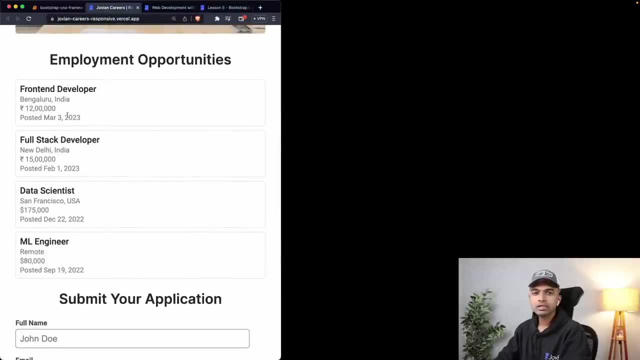 So here we are using a table on desktop. That is fine, But we will also see how to use cards on mobile devices, But right now we just have a list here. Yeah, so we are using cards of some kind here, but we'll see how to improve the layout of. 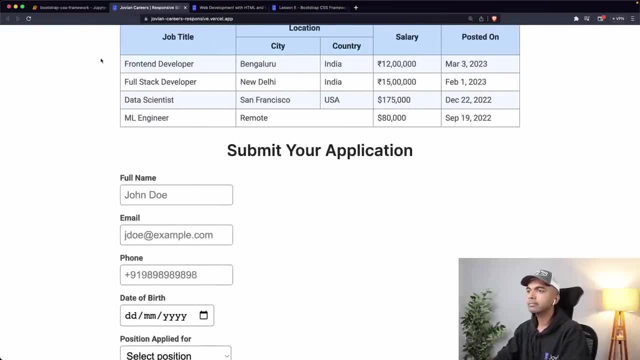 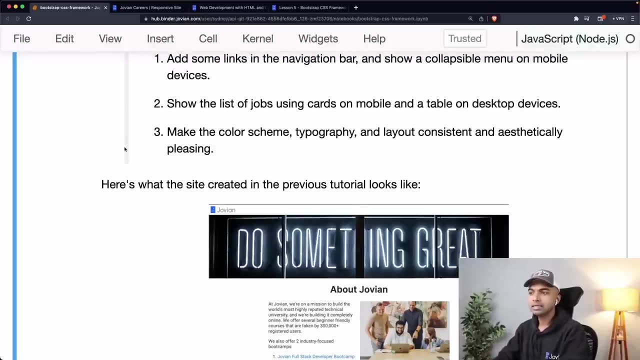 these cards using bootstrap, And we will also make the color scheme, typography and layout a little more consistent and a little more aesthetically pleasing. Okay, so this is the website that we had, and let's see what we're able to create today. 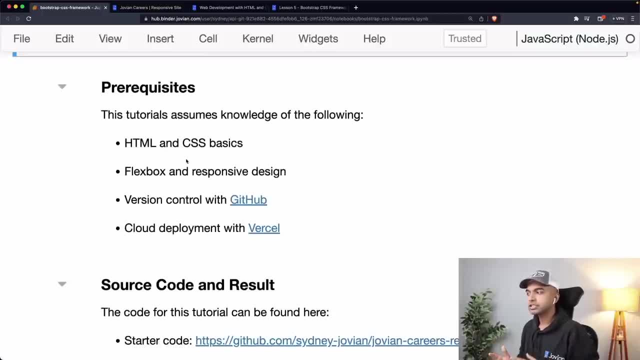 Now of course, we assume here, Okay, You have basic knowledge of HTML and CSS, And there is also an assumption here that you know about Flexbox and responsive design and version control with GitHub and cloud deployment to version. All of this is covered in the previous lessons. 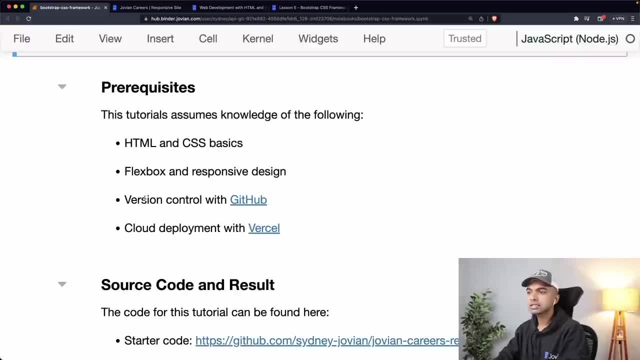 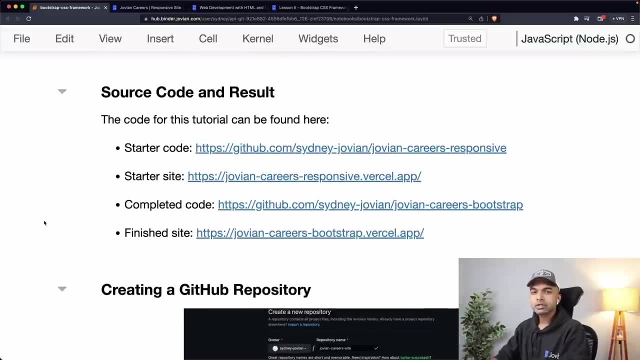 So I would highly encourage you to go back and review specific pieces If some of these parts don't make sense today. Now, please post your questions in the chat, because we will pause periodically and take questions, and the entire code for the tutorial can be found here. 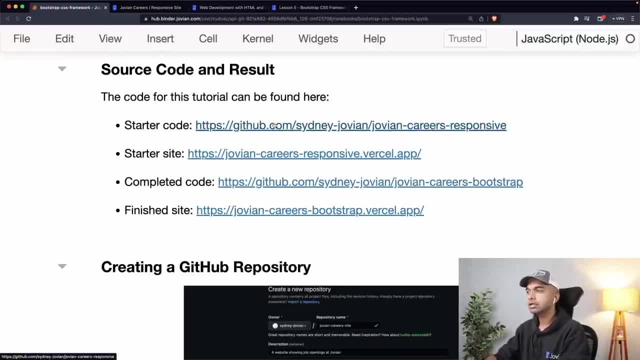 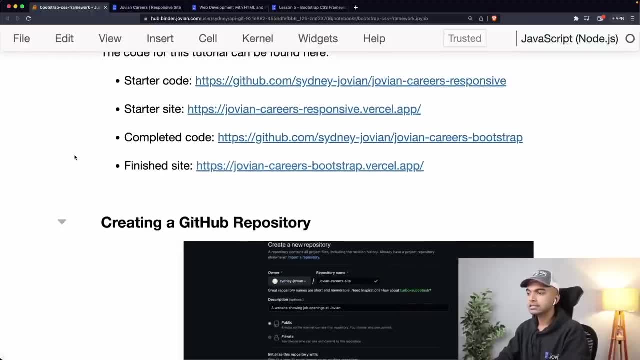 So the starter code, which is the site It created in the previous tutorial, can be found here, and the starter site can be found here, and you can find the completed code and the finished site using these links. So the first step today is going to be creating a GitHub repository. 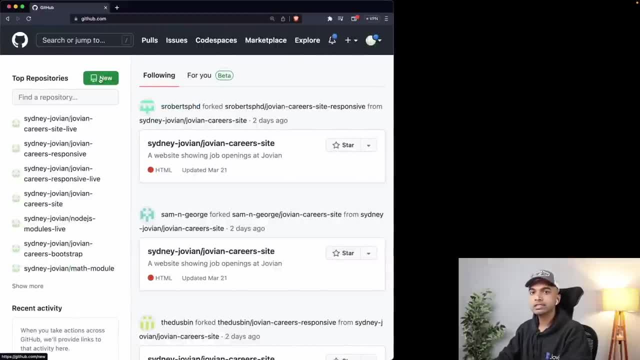 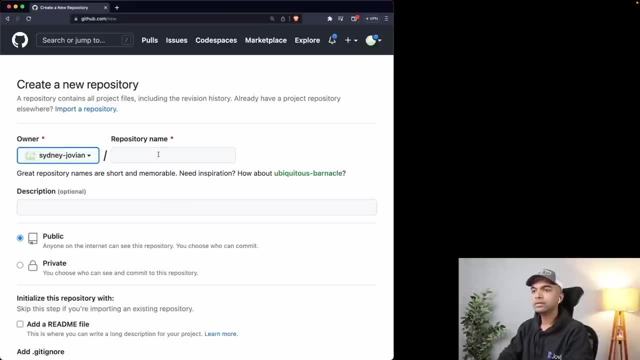 So I'm just going to go in here into githubcom And once I'm logged in I'm going to click the new button. And now I am going to give this a repository name, So let me just call it Jovian careers. 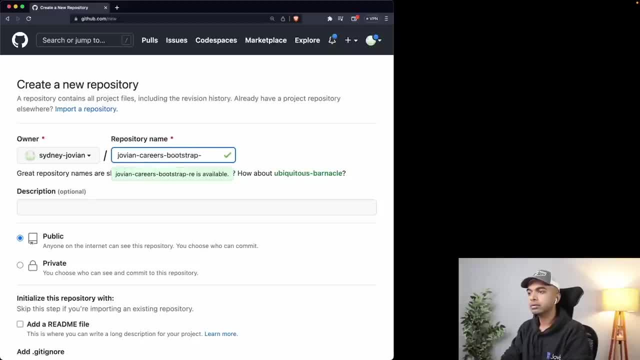 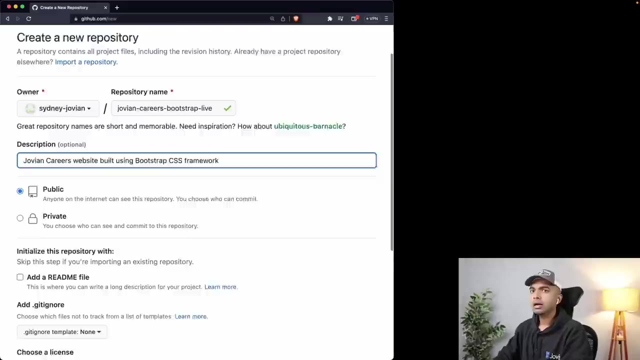 Bootstrap- Okay, Okay, So I'm going to give it a short description. I'm going to give it a short description: a Jovian careers website built using bootstrap CSS framework. I'm going to make this a public repository so that you can access this code when I'm 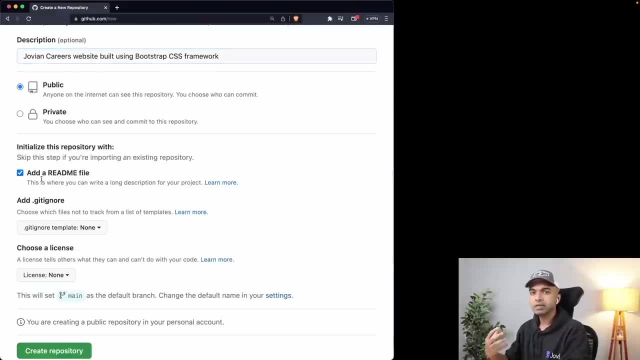 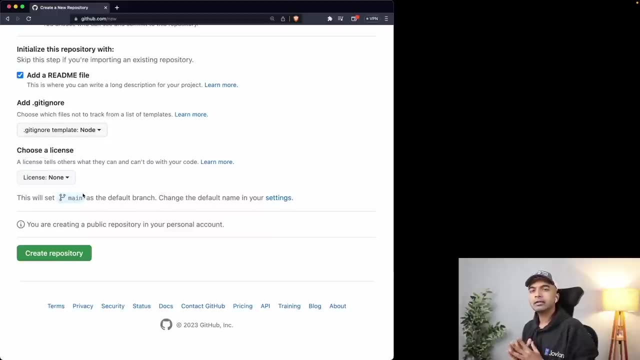 done. I am going to add a readme file as well, just so that I have some initial code in the repository. I am going to add a gitignore file as well, So I'm just going to type node, which is going to generate the gitignore file for JavaScript. 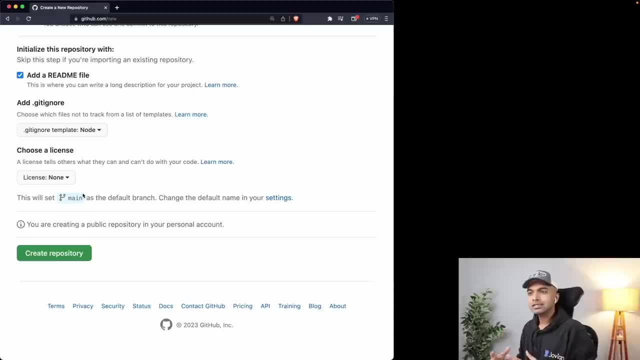 Which is going to ignore any files that are not necessary to be saved in version control, things like temporary files or compiled files, etc. And I'm going to add the MIT license here so that people can build on top of this. And now I'm going to hit create repository. 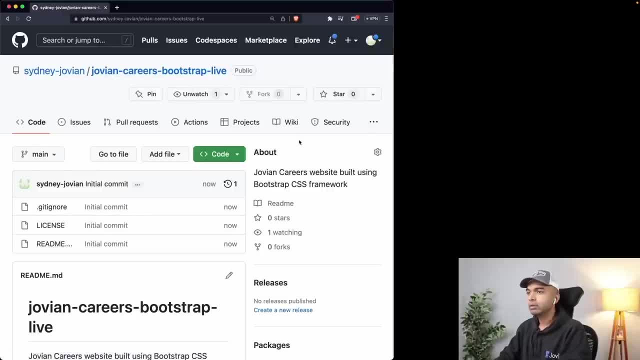 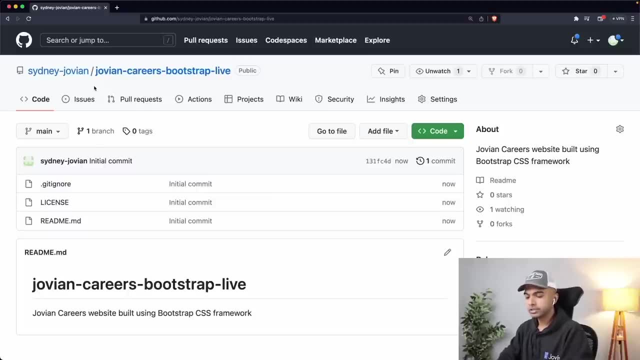 And with that, our GitHub repository is created. Perfect. So now we have a GitHub repository called Jovian careers bootstrap live And we now need to start developing this repository- Okay, Something that we'll do using code spaces. So we are going to use a cloud based programming platform called GitHub code spaces, which 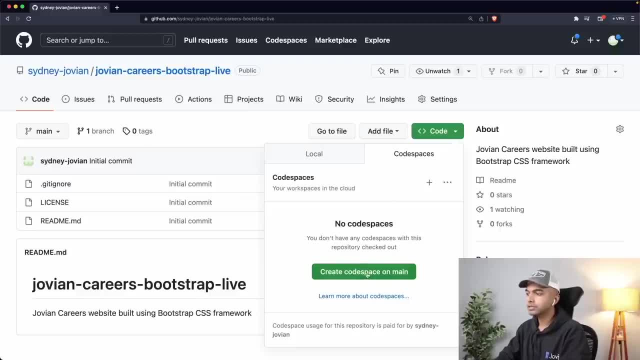 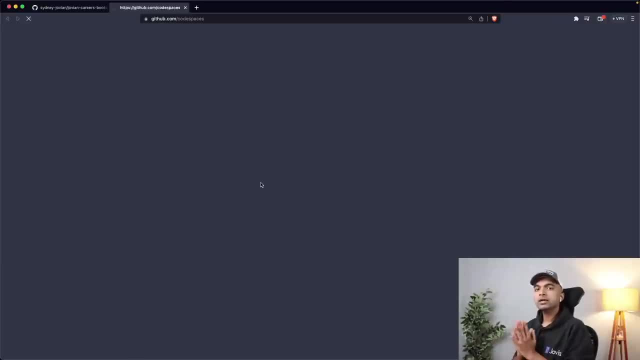 lets us open up VS code or Visual Studio code in the browser. So I'm going to just click the code button here and select create code space on mean, And that is going to now set up a new machine for us on the cloud. it is going to download. 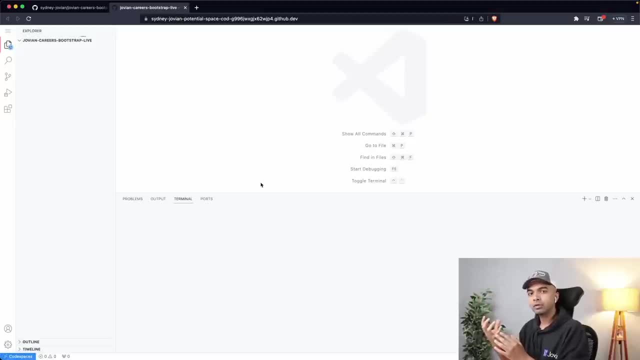 the code from the repository that we've just created onto that new machine, And then it is going to allow us to start developing it using this browser based VS code, And we can also start previewing it as we develop the website. Okay, So there we go. 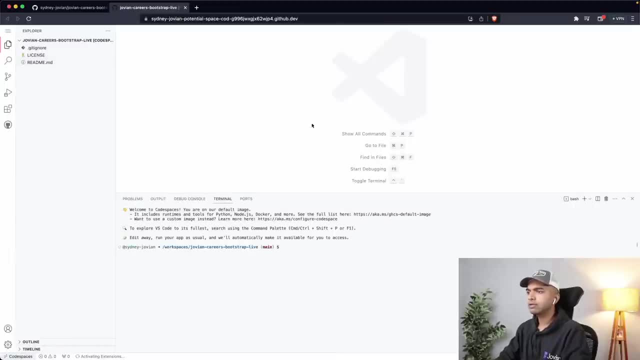 Now this has just opened up and I can open up any of the files here. And I can now open up any of the files here and start editing them. For example, I can open up the gitignore file here and start editing it. 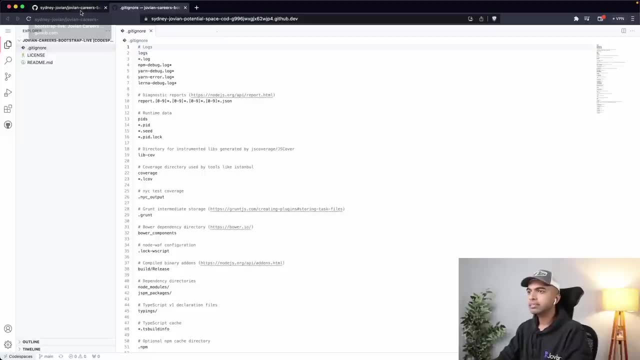 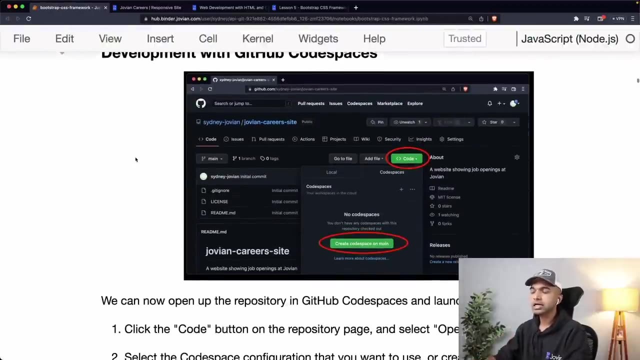 Okay, So with that, our basic development setup is complete. We have created a GitHub repository and we have opened it up using GitHub code spaces. The instructions are available in the notes if you need them. Now to begin, we can set up a basic HTML page. 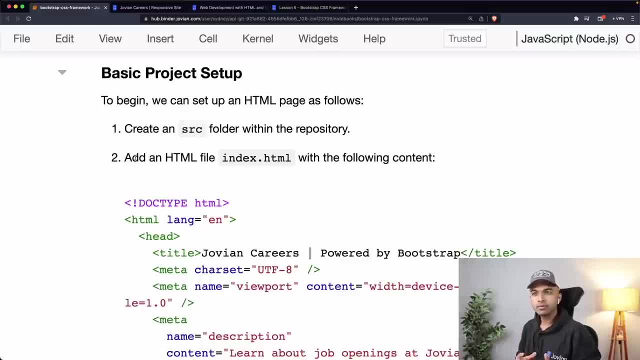 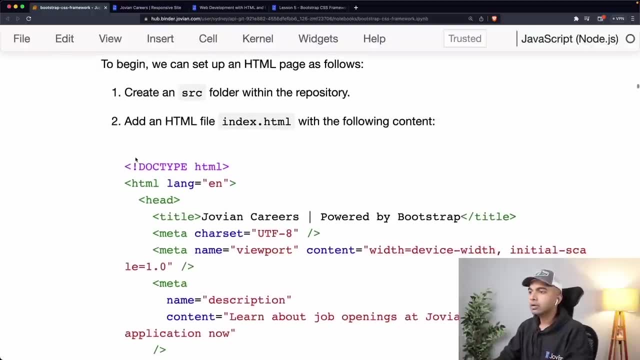 So we are not going to copy over any code from the previous tutorial. We are going to type out all the code, or most of the code, from scratch today. So let us create an SRC folder within the repository. It's always a good idea. 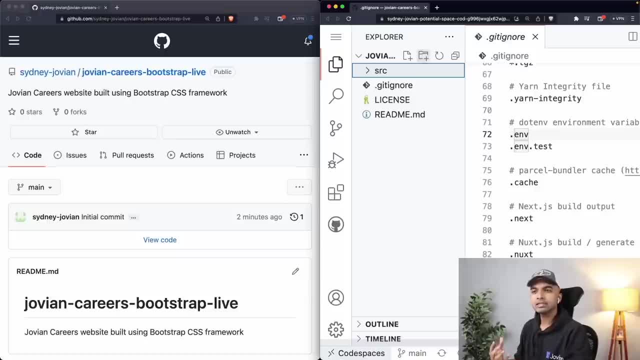 It's always a good idea to create an SRC folder containing the actual files for the project that are going to be deployed into production, because we don't want to send our gitignore license, et cetera into production. And in the SRC folder I'm going to create a new file, indexhtml. 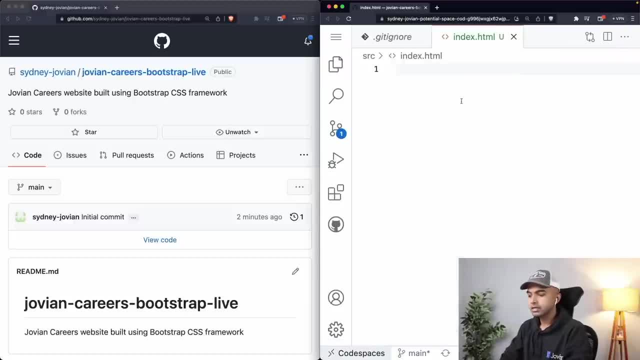 And now in my indexhtml I can start putting in some things. So I can start by, maybe, a doc type tag which just indicates that this is an HTML file. I can now go in and put in a head tag. Okay, Go in and put in a body tag and now I can start adding some information on the webpage. 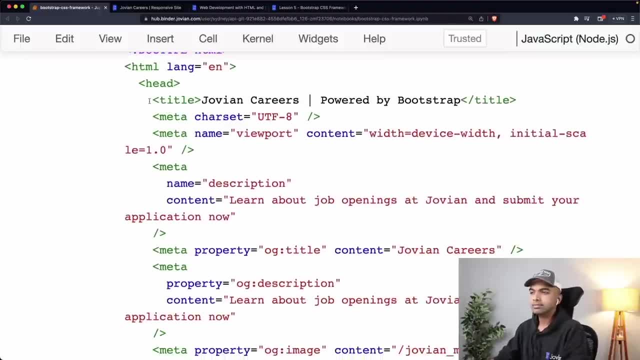 So I'm just going to copy over a few things here, which is something that we've been creating over the past few weeks as well. So I'm going to copy a title tag, So I'm just going to have this title tag in the head. 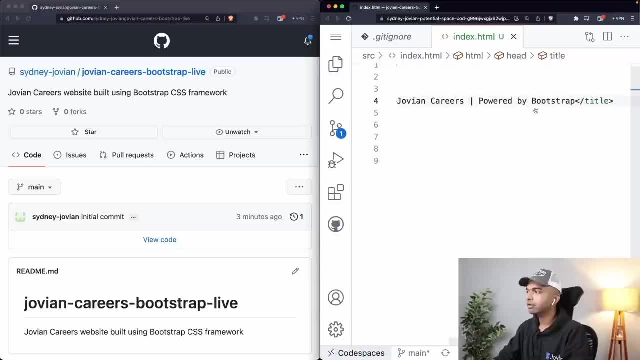 And this simply says that the title of the page is Jovian careers, powered by bootstrap. Then I'm going to copy a bunch of meta tags, Okay, And I'm going to add a tag to indicate to the browser that we are using the UTF eight. 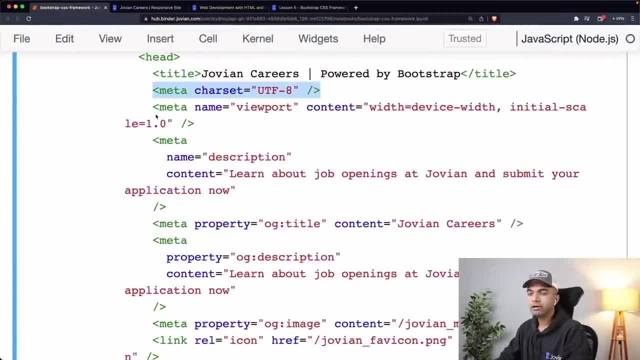 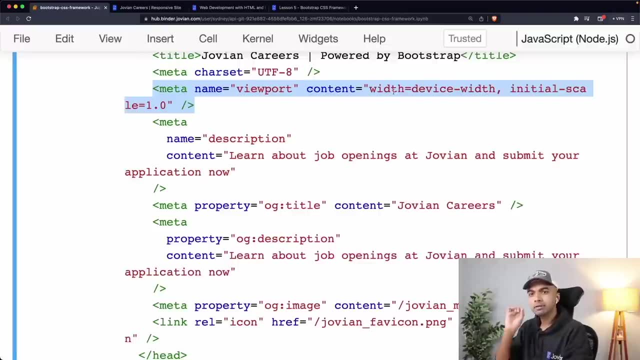 character set. So this is something that you should put into pretty much every website that you build. I'm going to copy over the meta viewport tag and the meta viewport tag, specifically with the content width equals device width and initial scale equal 1.0 is necessary for triggering. 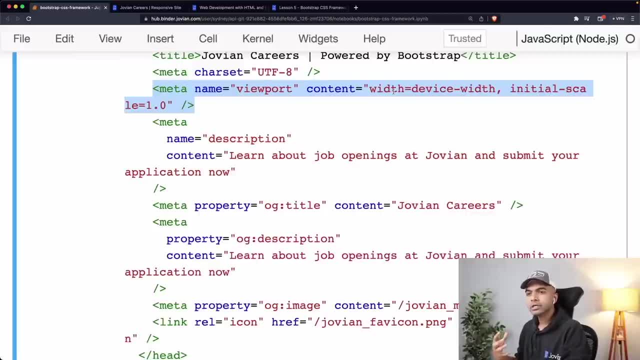 responsive design. Otherwise, older mobile browsers may try to automatically zoom in the content of your page, Like just for a desktop website. So this is a way of telling the browser that you have created a responsive design. Don't worry about what these specific things mean. 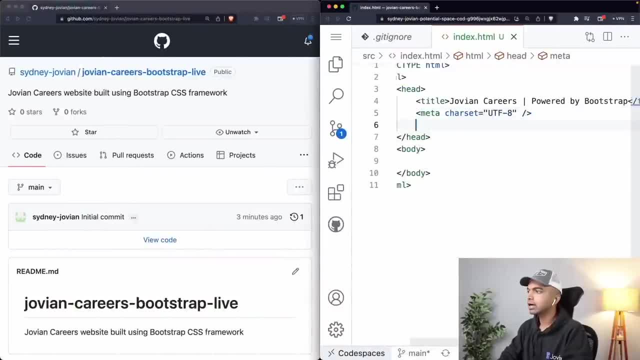 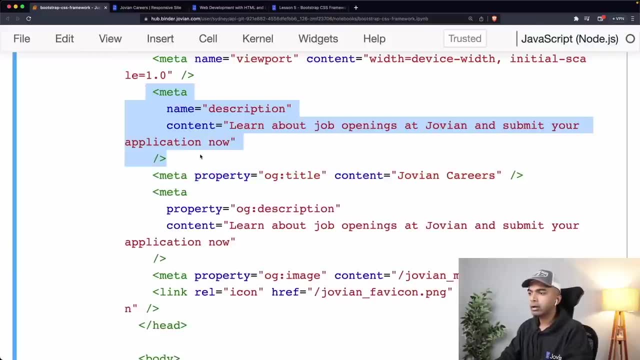 This is something that you should have in pretty much every webpage. I'm going to put that in here as well. Then I'm going to copy over a meta description and a meta OG properties. So an OG or open graph title, open graph description and open graph. 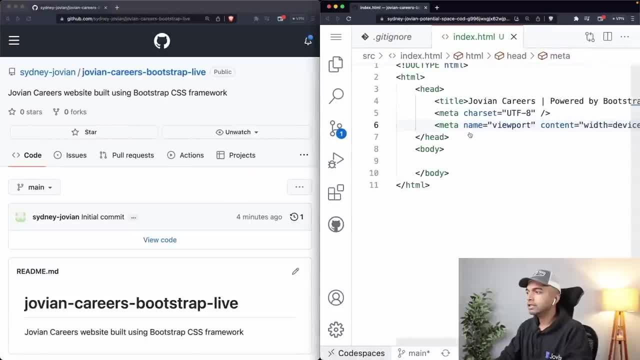 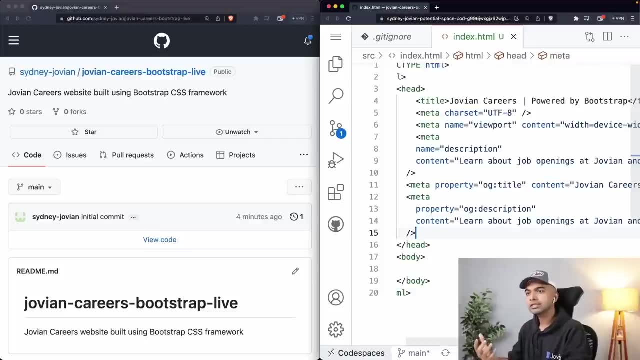 Yeah, Open graph description and normal description. All of these, as we've discussed in the previous lesson, Are used when you share the link that you have for the deployed web page with somebody else. So this is what. this is the title that is going to show up in the link preview. 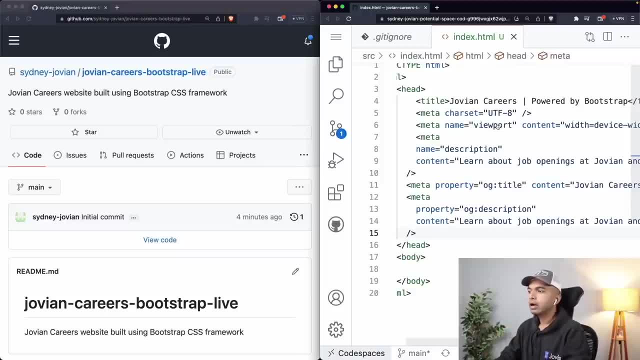 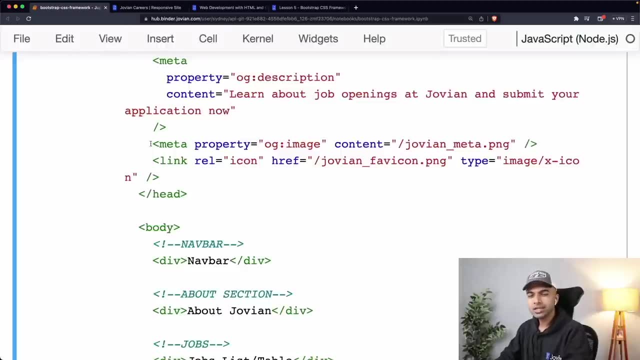 And this is the description that is going to show up below the link. Apart from that, we are also going to add a couple more tags, So there's going to be one meta tag called the OG image tag. This tag is going to determine the image that shows up as a preview image. 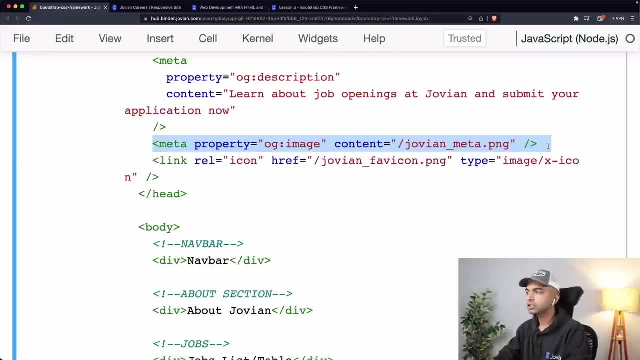 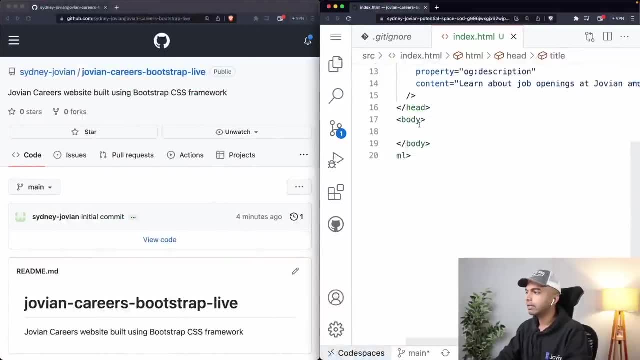 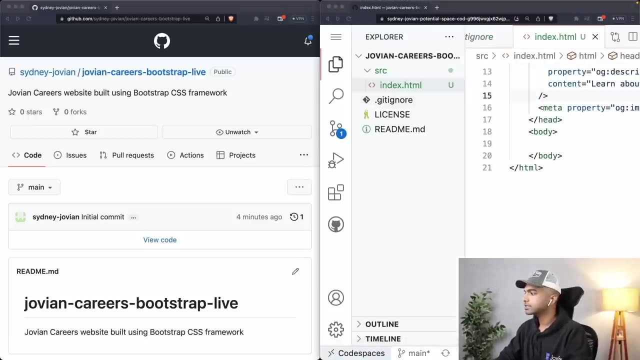 When you share this link on WhatsApp, Slack or any other social platform. and that is going to be something set to the Jovian meta dot PNG file And we're going to need that meta dot PNG file. So I'm just going to drag in that meta dot PNG file from my desktop. 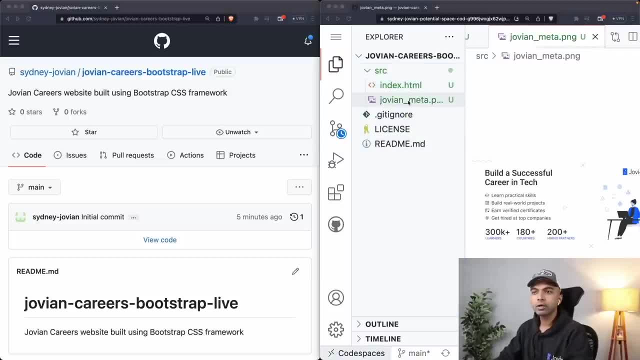 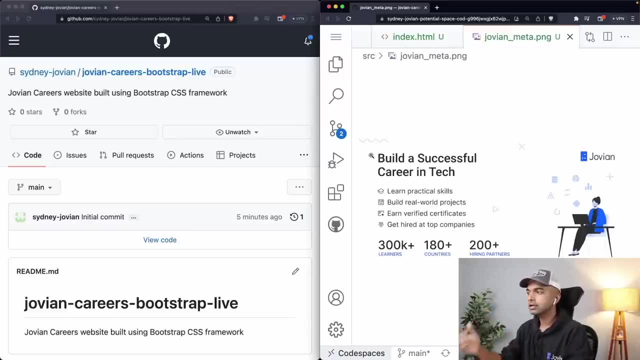 So I'm just going to drag in this file from my desktop into the SRC folder. So this is the file that is going to show up as the preview. This image is going to show up as a preview When somebody shares the link to our website online. 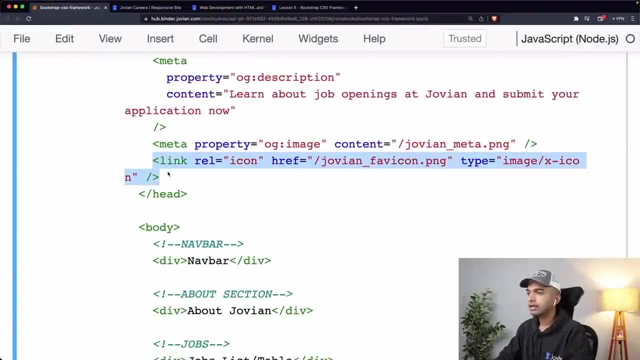 Okay, Finally, I am also going to drag a Put in a link tag with a rel equals icon, And this is going to point to the favicon. So the favicon is what is the icon? the little icon that shows up in the browser like this: 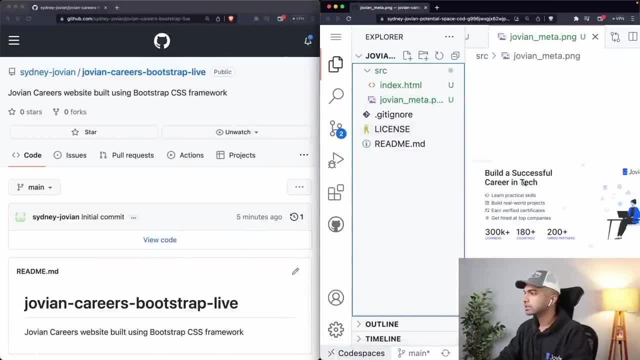 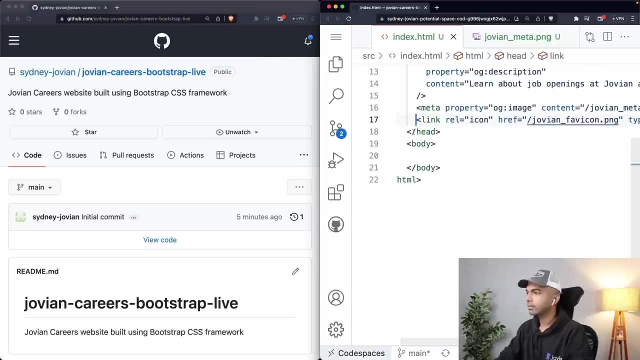 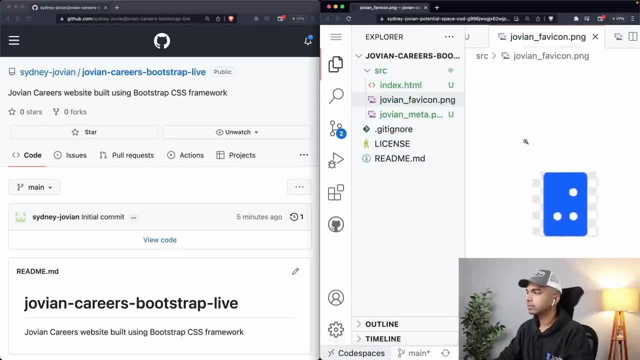 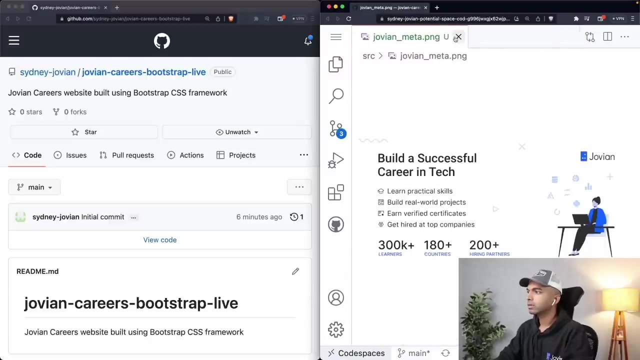 when we open that website in the browser. Okay, So let us add that meta tag in here as well. Let's add the favicon meta tag and let us bring that in here as well: Jovian favicon dot PNG. Okay, So with that, we have a basic setup of the page. 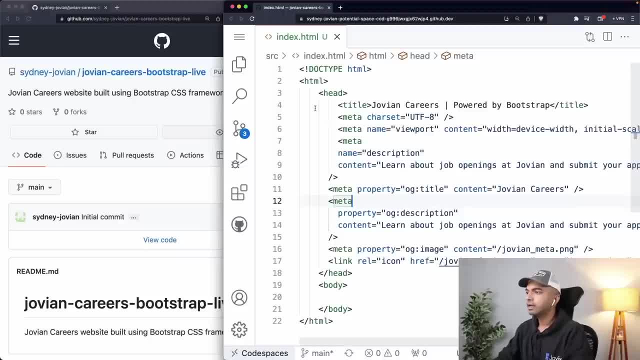 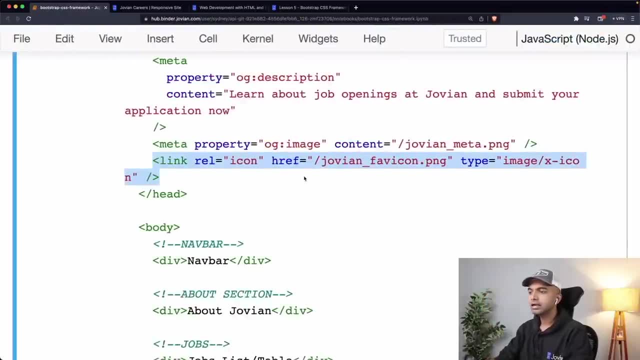 Let me just open it up here. So we have HTML, head title, meta, a bunch of meta tags. then in the body, because we are going to create this Jovian career site, I'm just going to put in a bunch of empty. 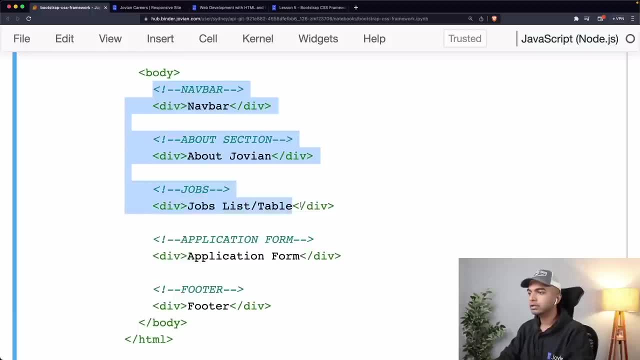 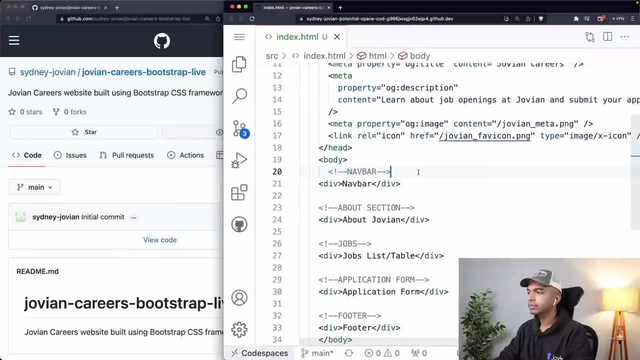 divs for now. So I'm just going to put in a nav bar and, about Jovian div, a jobs list and application forms. All of these are just empty. I'm just going to put in the divs along with HTML comments about them. 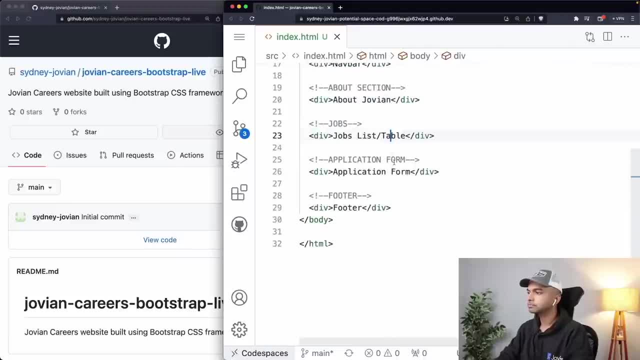 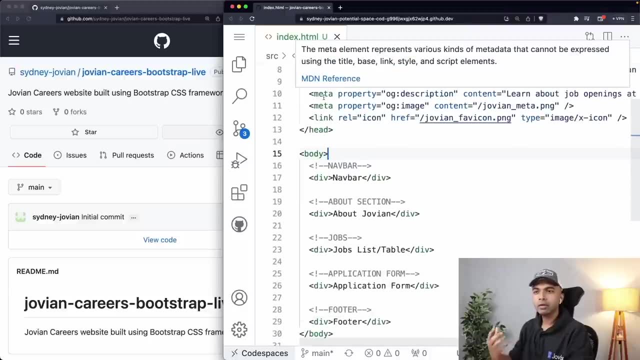 So let's do that as well, And let us just format the document. Okay, Looks good. So now that we have some code that we have added into our HTML page, we need a way to actually see what this page looks like, And that is where we're going to use the live server extension. 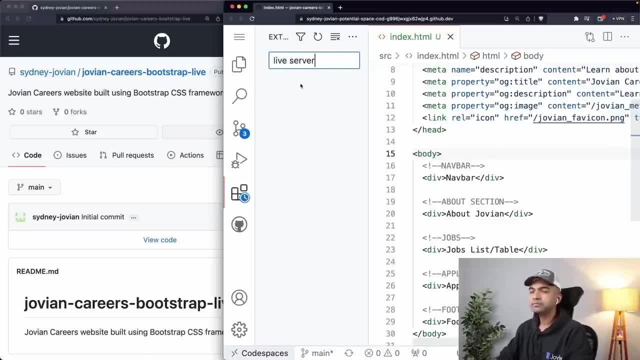 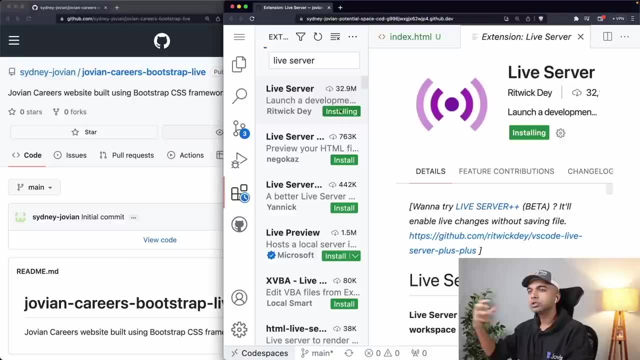 So I'm just going to search live server And the live server extension allows us to preview the webpage that we are building in our code spaces machine Which is running somewhere on the cloud. So it sets up a server and it serves that page so that we can open it on the browser. 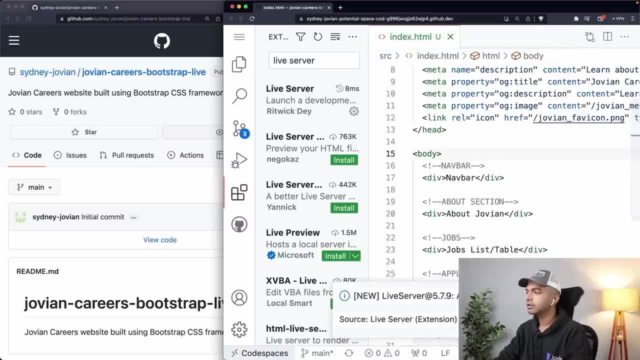 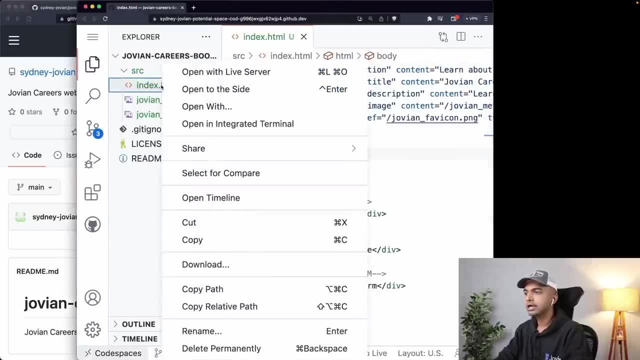 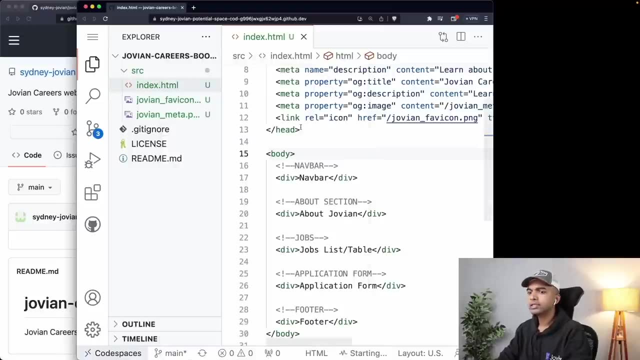 And once it is installed I can come back into my indexhtml file And right here at the bottom I should be able to see a go live button. or I can also just right click on my indexhtml file and just select open with live server. either way, 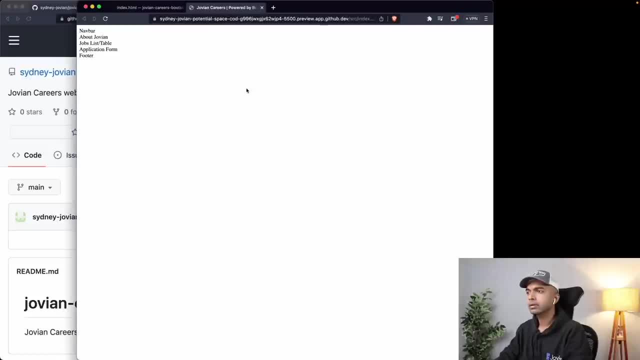 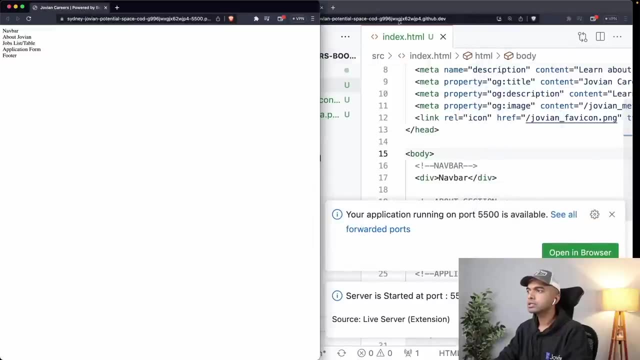 Once I click this, you can see that the website is open. Okay, Okay, So the website is now open, All right. So let me just put that website here. So this is a site that we have right now And this is a site that we are going to start slowly building. 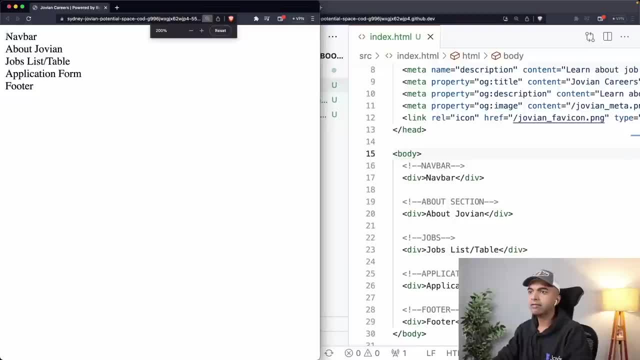 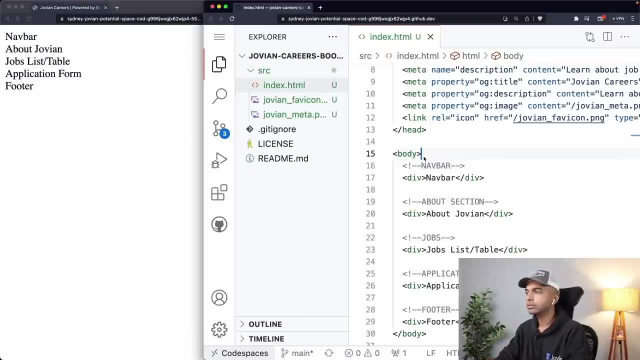 You can see that there's not a lot here, Even if I zoom in there. there is just this navbar. There's a bunch of divs with some placeholder text within them, And this is a site that we are going to slowly start building using bootstrap. 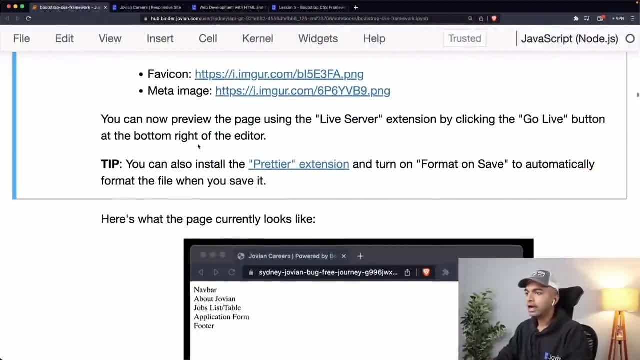 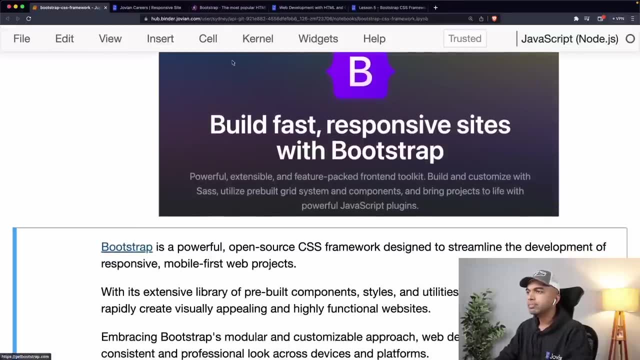 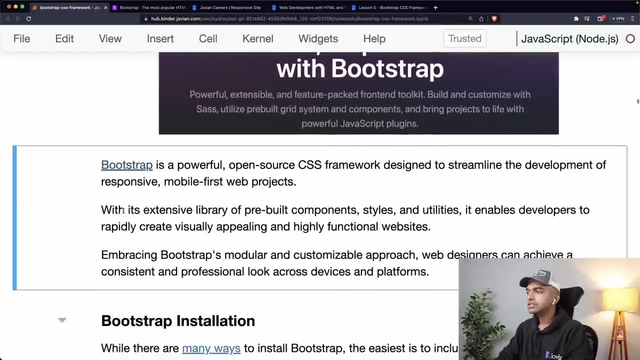 Now, with that out of the way, we can start Actually using the bootstrap CSS framework. So bootstrap is a powerful open source CSS framework And this is the website of bootstrap: getbootstrapcom. It is designed to streamline the development of responsive, mobile first web projects. 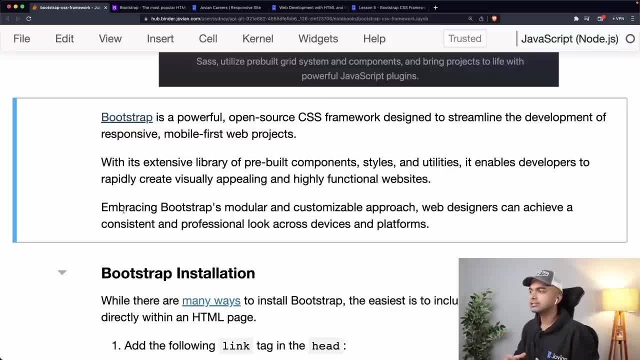 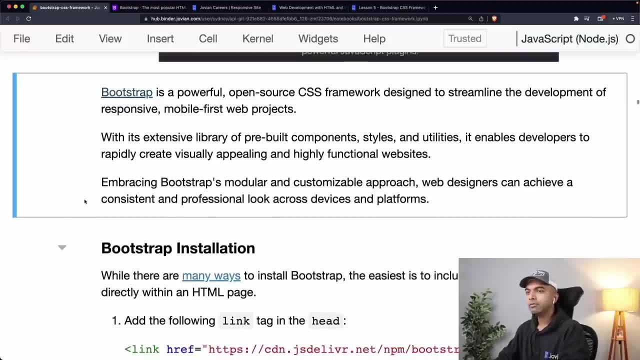 And it has an extensive library of prebuilt components, styles and utilities, and it enables developers to rapidly create visually appealing and highly functional websites, the Lord of the websites that you see on the internet. Either use bootstrap or something else. Okay, So bootstrap is something very similar to bootstrap, some kind of a CSS framework to 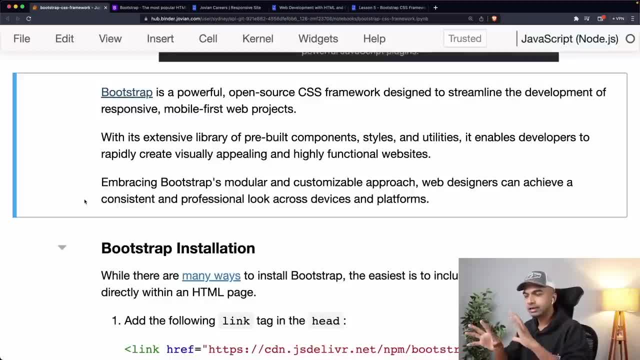 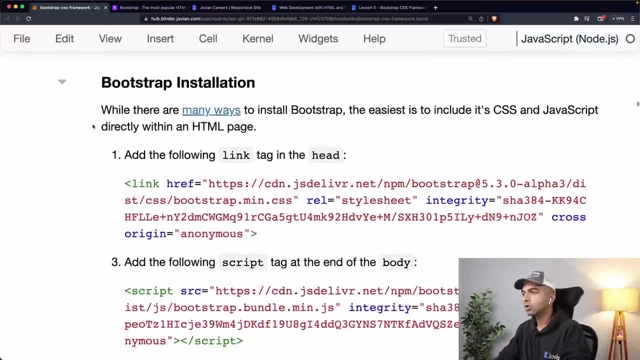 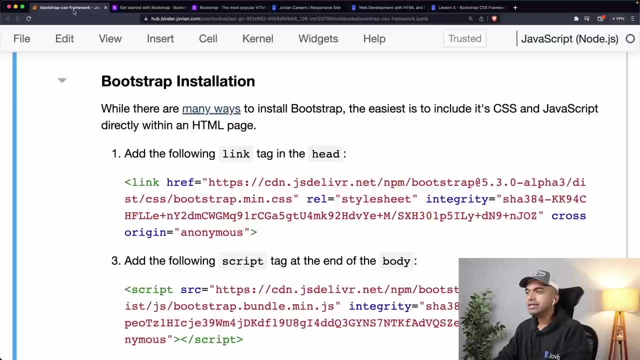 add all the interactive features, all the various interesting layouts that you see on most modern websites. And there are many ways to install bootstrap and you can check out the different ways of installing bootstrap on the website on the get started page. But the easiest way to use bootstrap is to include it CSS and JavaScript directly within. 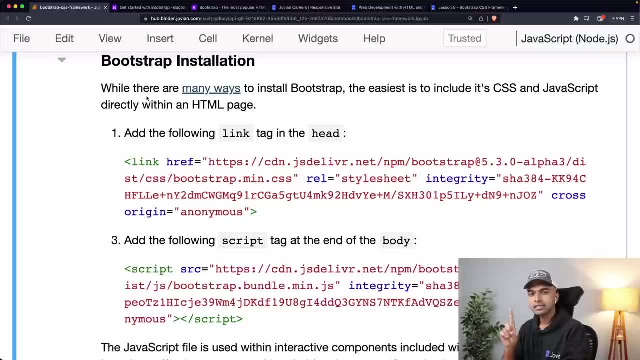 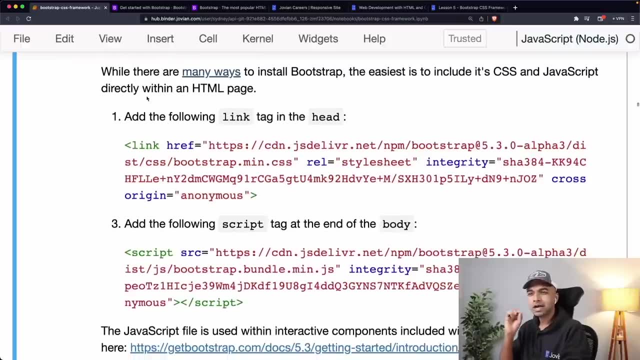 an HTML page. So bootstrap has two parts. It has the CSS file, Which contains a bunch of existing styles that you can use within your HTML page, And it has a JavaScript file. JavaScript is used to enable some interactivity, things like dropdowns, popups, tooltips, etc. 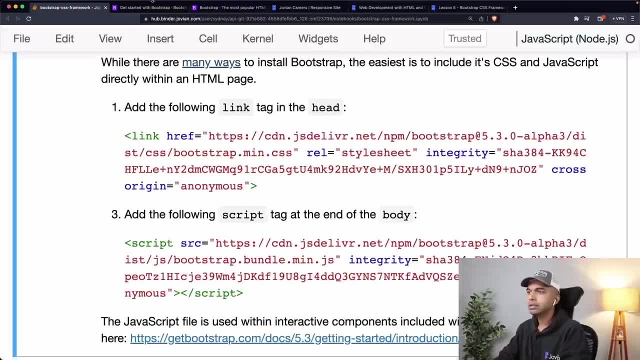 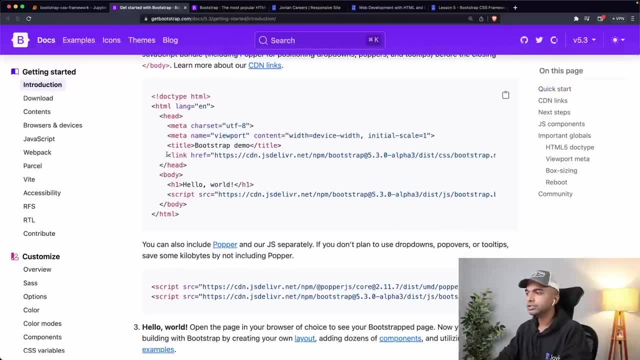 So there's a JavaScript file that you need to include as well. Okay, So let us first grab the link tag. So there are two things here. There is this link tag right over here, which contains the bootstrap CSS file, So I'm just going to grab that. 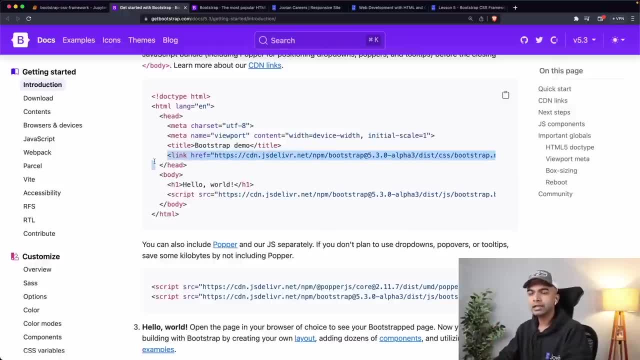 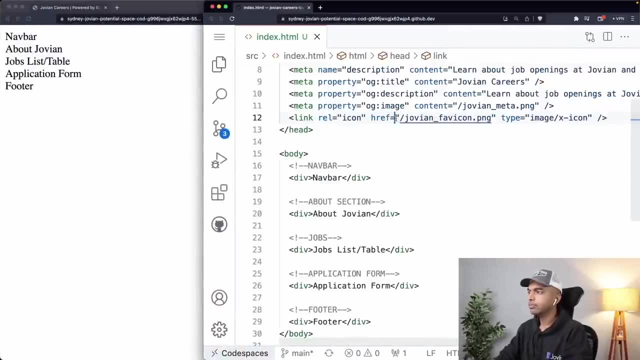 And it's always a good idea to grab it from The website, because that is going to have the latest version of bootstrap, which currently happens to be 5.3.0.. So I'm just going to come in here and I'm going to paste this link tag right here, right. 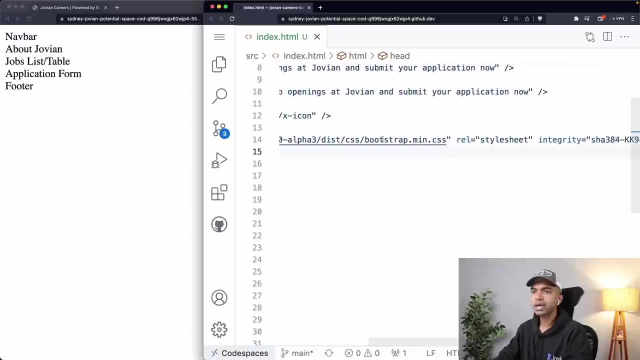 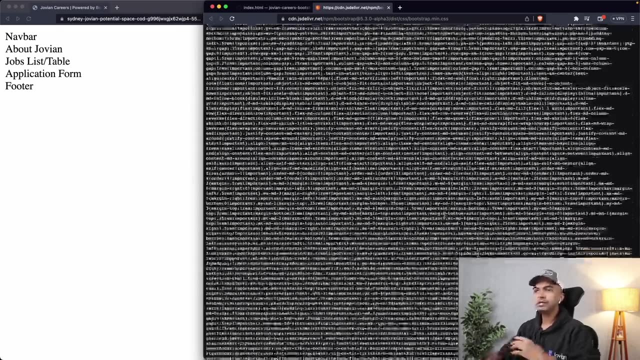 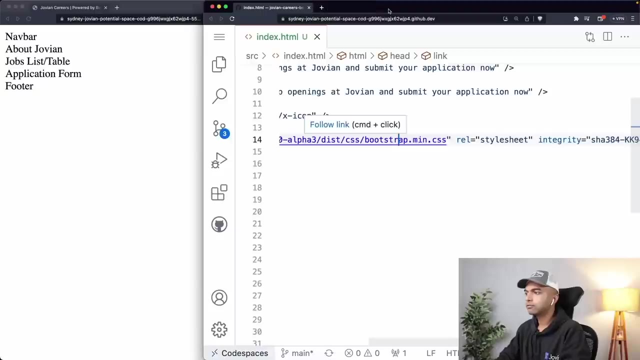 below You can see we now have this link tag bootstrapmincss. that gets included, and you can also command: click this link and see what that file contains. So you can see that it contains a whole bunch of CSS styles. We will obviously not be using all of them, but many of them are going to be useful for. 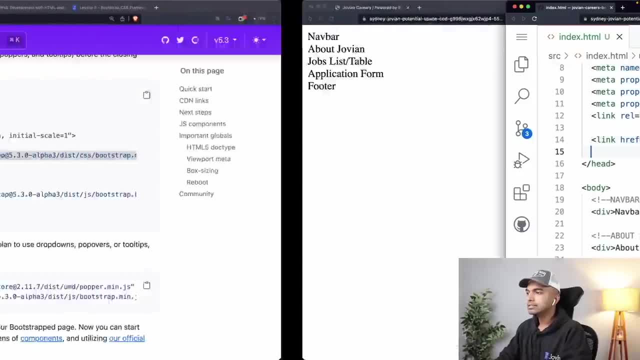 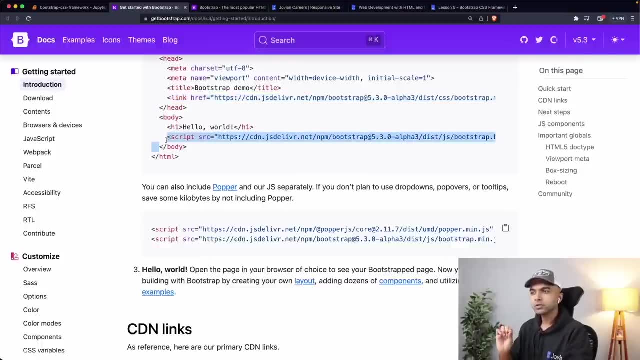 what I'm going to do today. Okay, So that is the link tag. Then another thing that you can do is include this script tag, And interestingly, the script tag goes not in the head but in the body and right at: 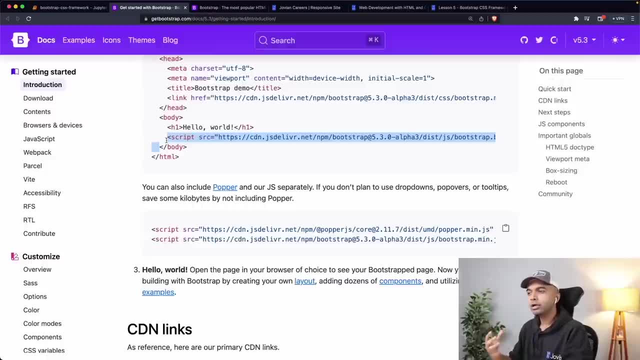 the bottom of the body, And the reason for this is you do not want the loading of the script to prevent or block the loading of the webpage, And that is why putting it, the putting it at the end of the body, ensures that only after 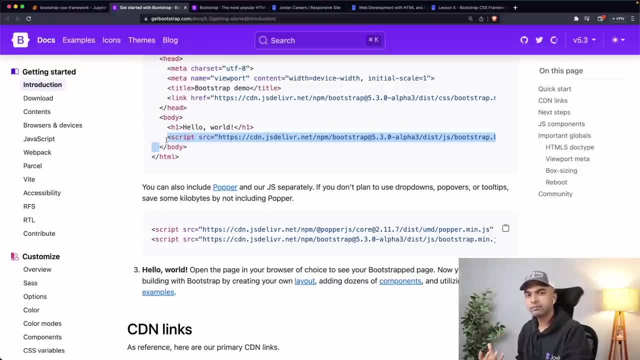 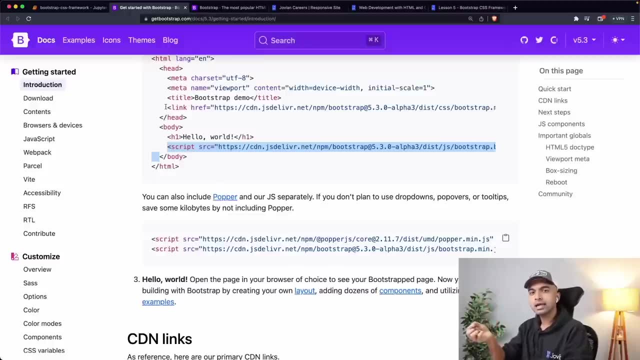 the entire content of the HTML page is loaded. only then the JavaScript file gets loaded. Okay, We don't do that for CSS, because we want the styles to load beforehand. Otherwise, if the store styles load after the page loads, there's going to be a flickering. 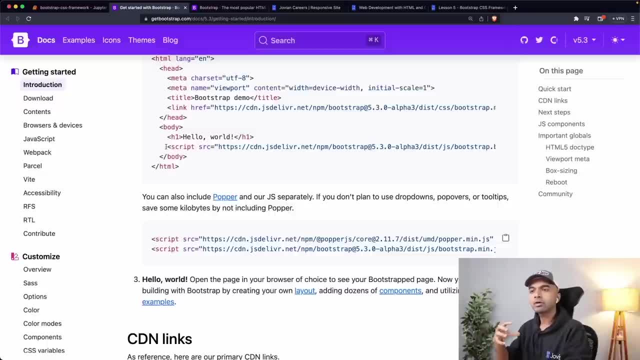 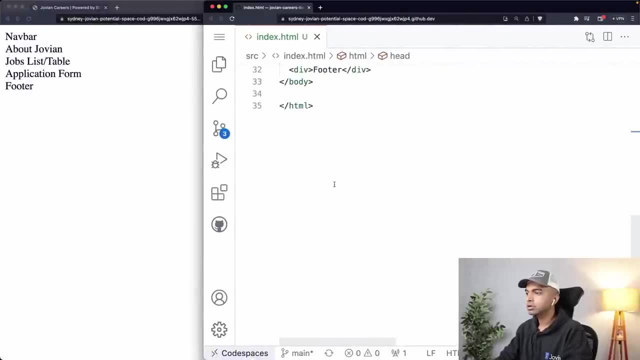 effect. but for the script, because a lot of the interactivity is going to happen after all the content loads, it is okay to put that script at the bottom of the page. Okay, So I'm just going to go in and put that script right at the bottom of the page. 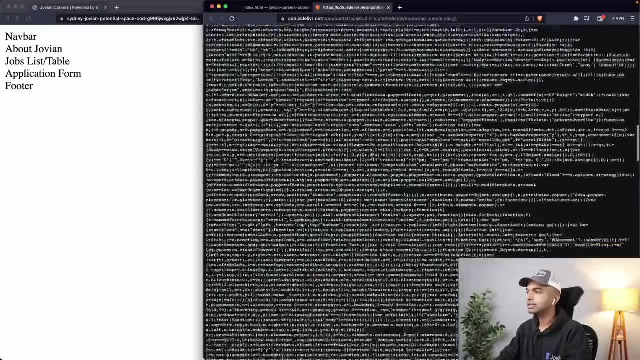 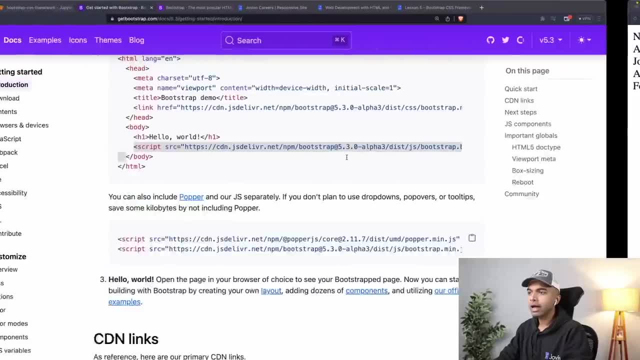 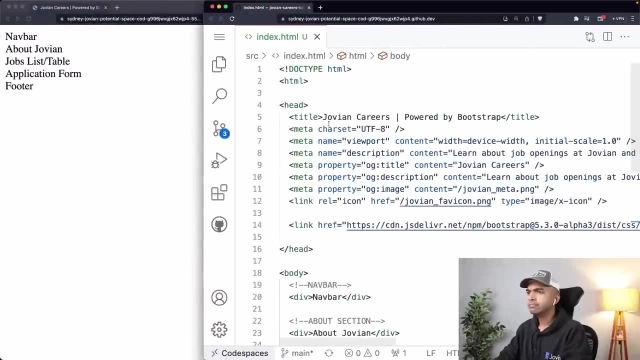 And you can see again. there is this: bootstrapbundleminjs, and this is all the JavaScript that is getting included by default. So that is how you add bootstrap to your webpage And once you save the file and come here and reload the page, you can see already that 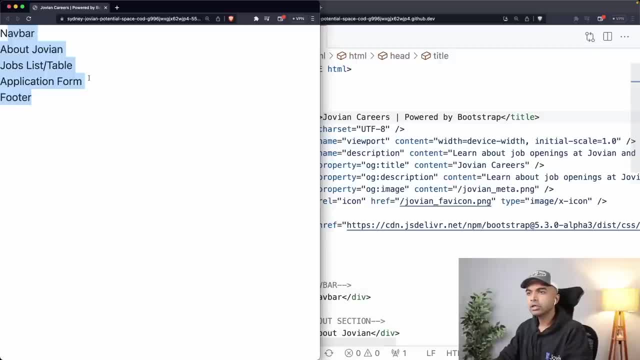 the styles have changed significantly. So earlier we had a slightly different font. We also had some default padding. but let's say- I comment this out- You can see that there is some padding on the body. You can see that the font is slightly different. 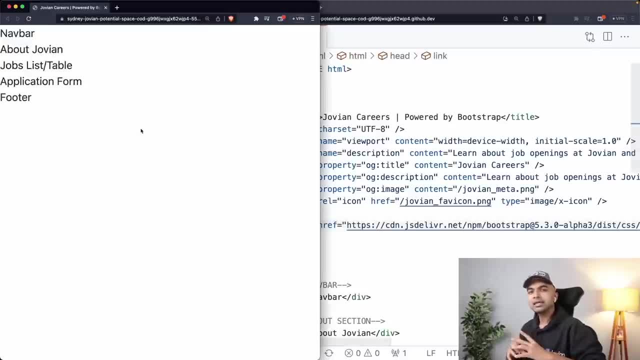 So there's already some change that bootstrap has brought in. In fact, it resets a lot of the basic styles and it sets up basic styles for text. It sets up basic colors for the text, It sets up basic font sizes, fonts. It sets up a bunch of things by default. 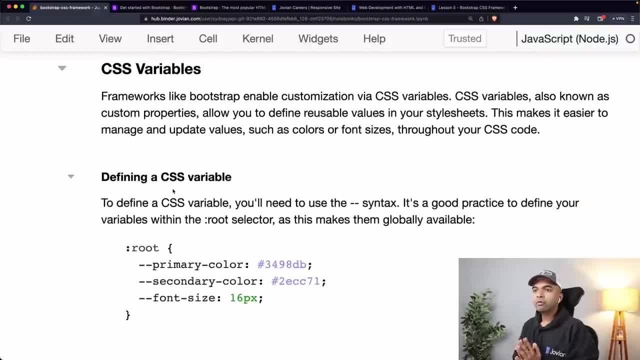 So that is how you set up bootstrap. Now, before we actually start building something, we will have to start first. maybe customize the bootstrap setup to use the fonts and the colors that we want to use, Because, given the Whatever company you're working at, they're going to have their own preferred fonts and 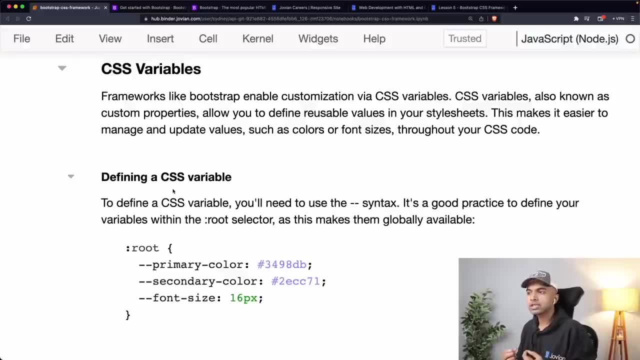 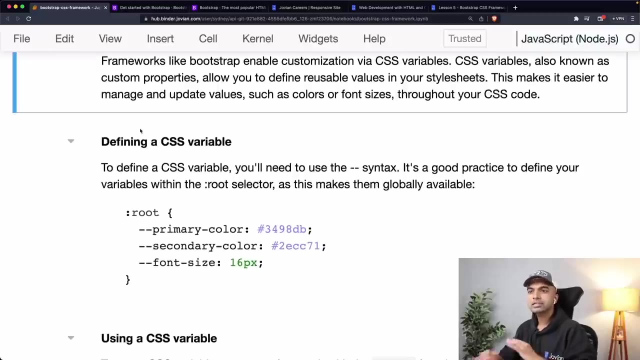 colors that you might want to use, And you can override or customize bootstrap very easily, And frameworks like bootstrap enable customization via CSS variables. And CSS variables, also known as custom properties, allow you to define reusable values in your style sheets, And this makes it easier to manage and update values such as colors and font sizes throughout. 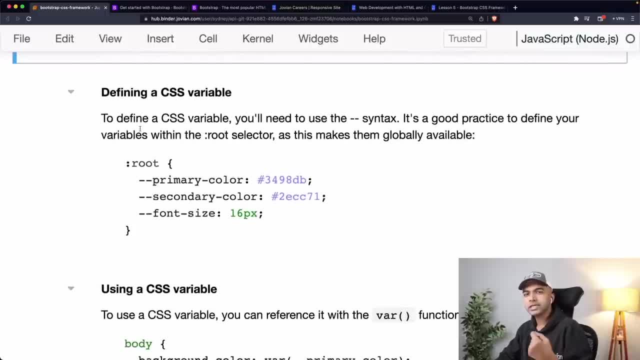 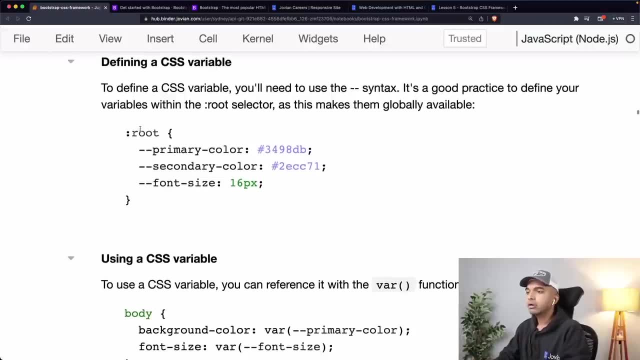 your CSS code. So I'm going to give you a quick tutorial of CSS variables and then we're going to start customizing some CSS variables to change what bootstrap gives us. Now, to define a CSS variable, you need to use the hyphen, hyphen syntax or the minus. 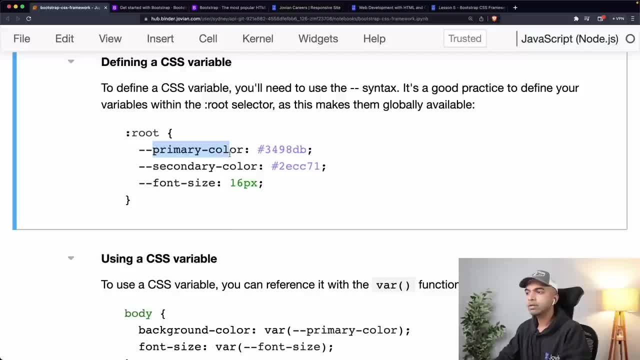 minus syntax. So anytime you put minus minus followed by something that is treated as a CSS variable. That's the first thing. The second thing is, as a good practice, you should always define your CSS variables in this selector called colon root, And this is just. 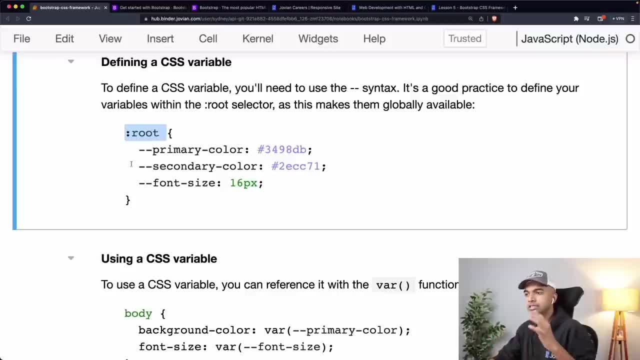 This is called a source. This is a pseudo selector. This basically says that you want to put these variables- and you want to make these variables available- right at the very root of the CSS file, so that it's available no matter where you are in the CSS file. 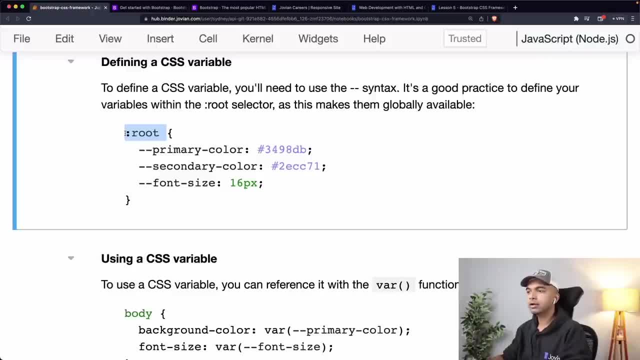 Okay, So it's it's. it'll be at the root of the document and it'll be available across all different kinds of styles, Maybe even inline styles and style tags within the page. So here is how you can create some CSS variables. 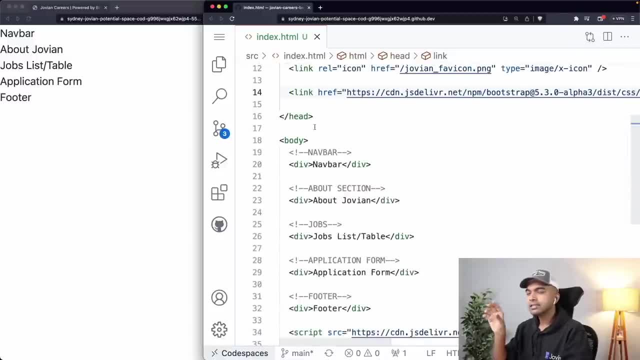 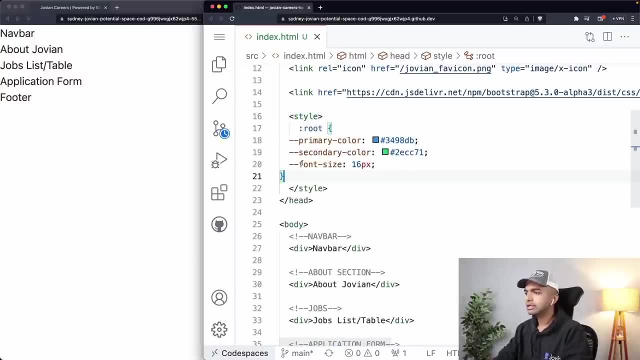 So right now we don't have a CSS file that is con, that is connected to this webpage, But I can just put in a style tag here for now And I can just create a bunch of CSS variables here using the root tag. Okay, 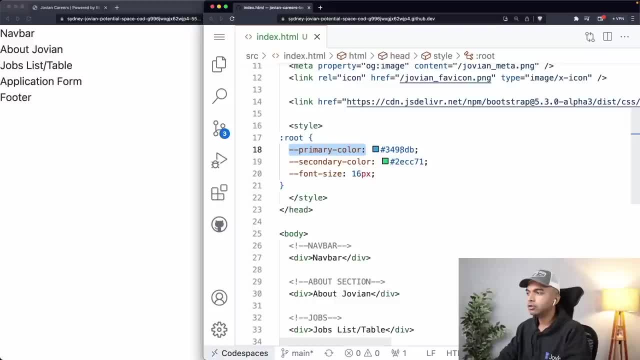 So now I have this root, and in the root I have set a primary color to be a certain blue, I've set a secondary color to be a certain green and I've set the font size to be 16.. These styles are not applied to anything yet. 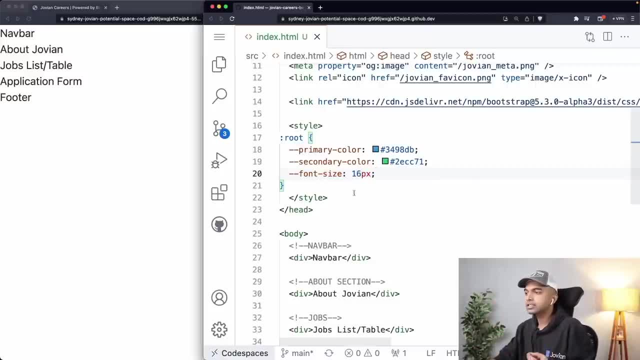 These styles are just variables, So just like variables in any other programming language. the hyphen hyphen font size is a variable. It has the value 16 pixels. and similarly, hyphen hyphen primary color is a variable. It has the value blue or a variation of blue. 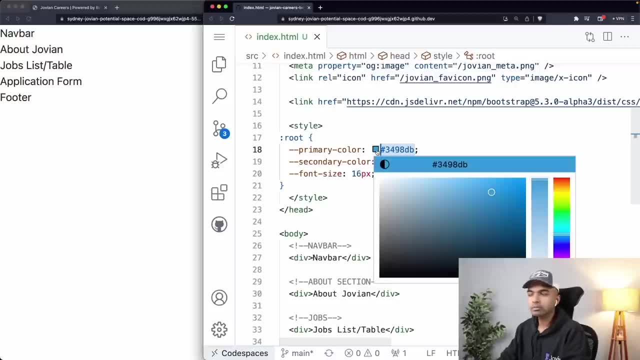 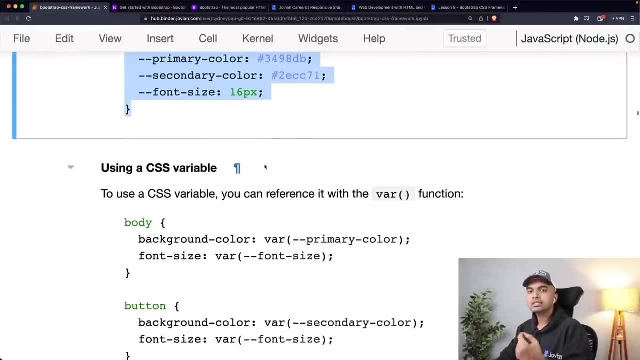 Okay, And of course, this is the hex code of the color and VS code show very helpfully shows us a preview as well. Now, once you've defined a CSS variable, you can then use it within some CSS property, and you can use it using the var function in CSS. 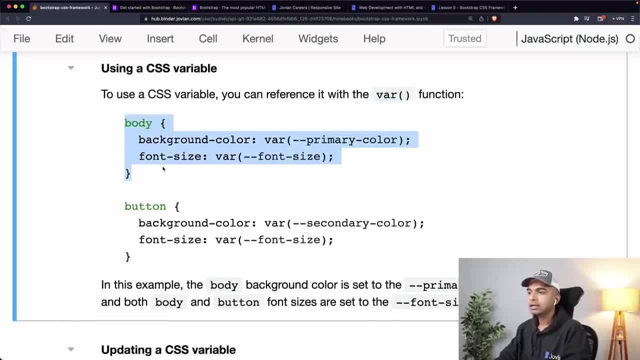 So here is how you might use it. You might say something like body, and then you might set the background color of body to var. And then here you provide the name of the color, provide the name of the variable hyphen: hyphen primary color. 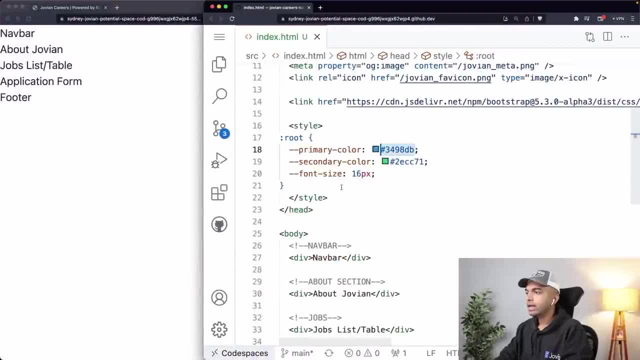 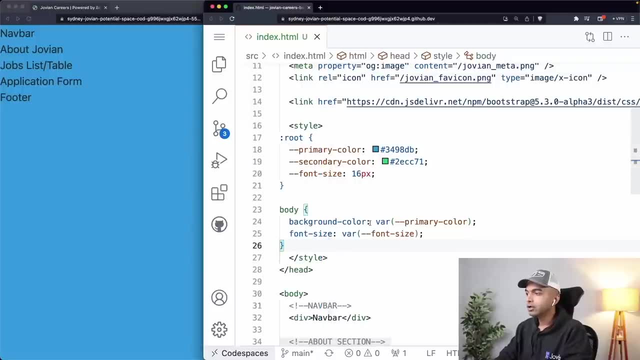 And now what's going to happen is, when I paste in the style and I save the page, you can see that the body got a background of blue. That's because var- primary color- invokes a search for CSS variables And there is a CSS variable in the root called primary color, and its value has been set to. 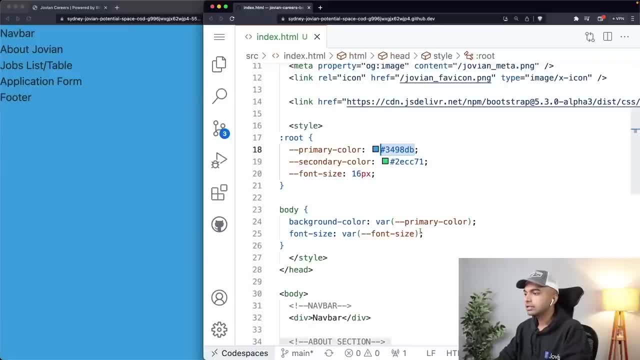 3498 db, which is a blue. Similarly, the font size of the body is going to search for the variable font size and that is going to get the color 16.. Now, the benefit of CSS variables is you can now go in and you can actually update these. 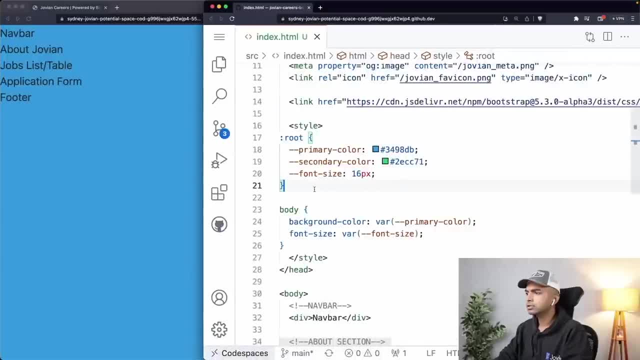 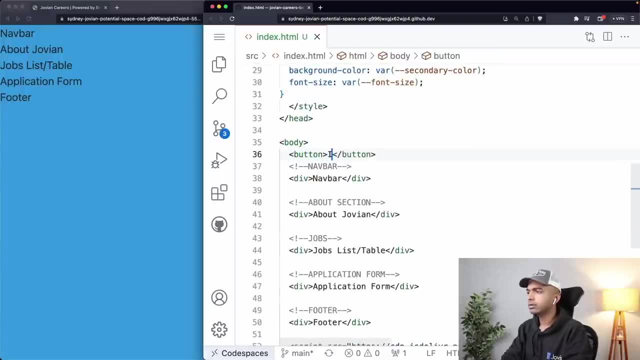 variables. So, once again, if I go in here and then let me also create a button here just to complete this example, And let's put a button right here, right at the top, Let's say click me, Let's say that there's a button right here, right at the top. 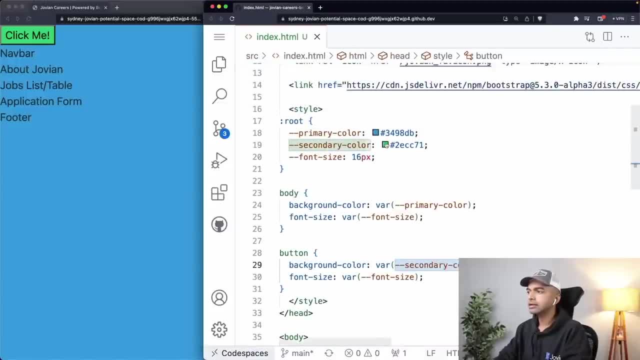 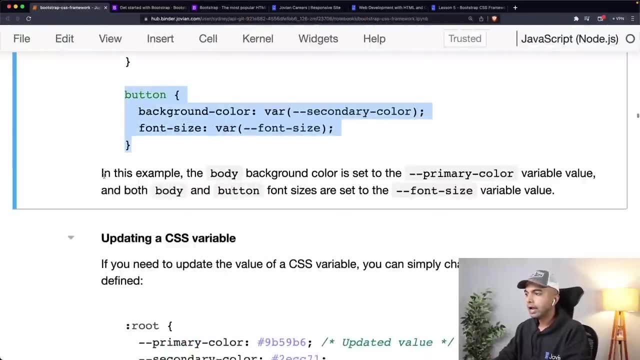 And this button has the color secondary color, and the secondary color is a green. So clearly, the button has a green color and the CSS of the body has a blue color. Now you can go ahead and update a CSS variable, So you can either update it at the same place where you defined it or you can update it. 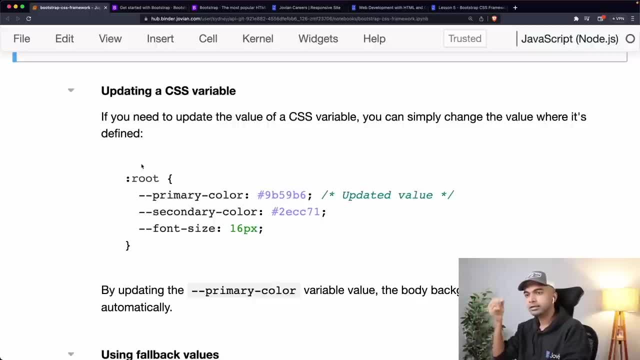 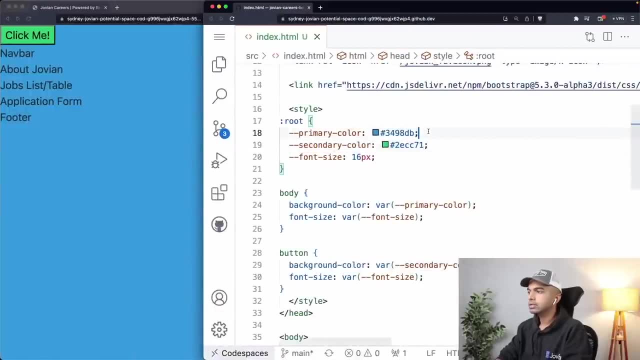 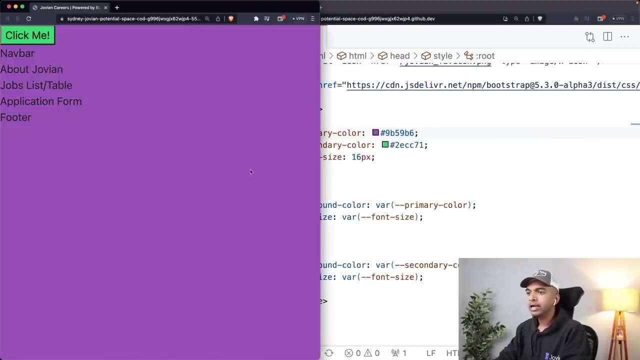 somewhere. Maybe. let's say you have a bunch of CSS files and you've updated it in a second or third file, So let me just go in and update these two values. I'll just update the primary color And now you can see, as soon as I update the primary color to a purple, that automatically 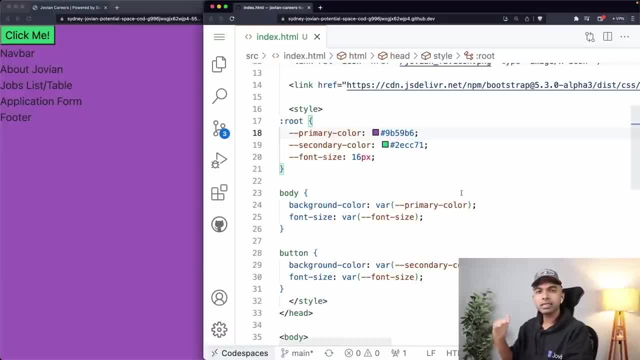 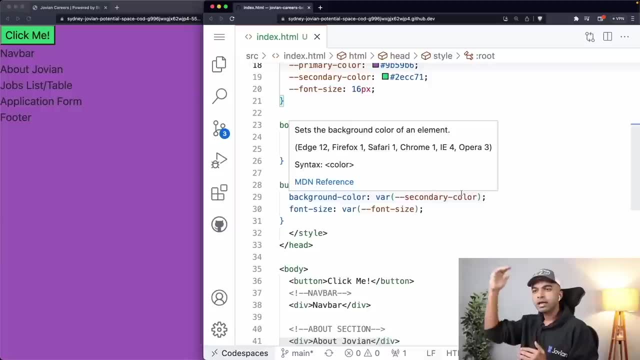 updates the background color. So wherever the variable is used, the color is now going to get updated. Okay, so now you can see the value of CSS color CSS variables. I can define a bunch of variables based on the theme that our design team has currently given us, that I can just. 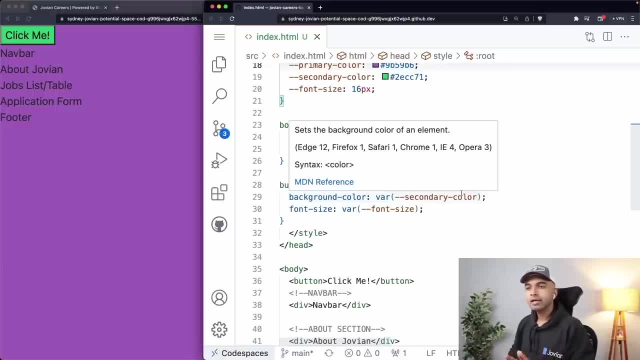 use those variables everywhere in my CSS styles And then when the design team comes in And says, Okay, we need to change the color. we are moving from blue to red. we don't have to go in and edit a bunch of different properties. 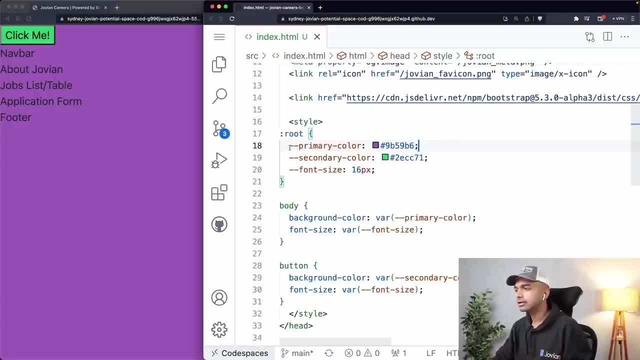 We just go to our root tag, our root selector. we just simply check the primary color and change its color to whatever the design team is asking us to do. Okay, so that is the value in CSS colors, So that is a value that CSS variables provide us. 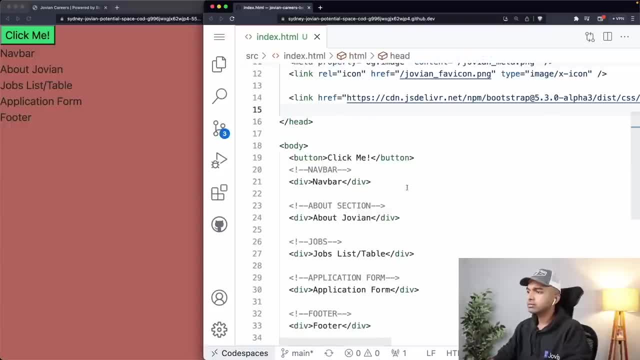 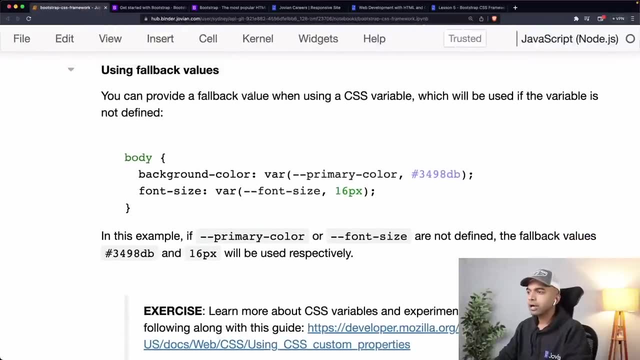 Okay, So for a moment, I'm just going to get rid of all of this now. now that we understand how CSS works, The last thing you can also do is you can also provide a fallback value So that, let's say, you're providing a background color and that is going to come from a variable. 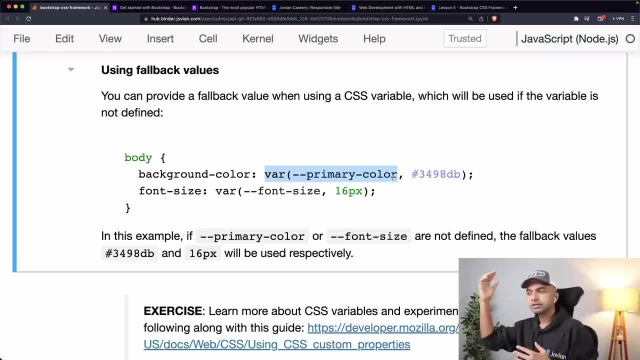 Let's say this variable is not defined. for whatever reason, somebody went and changed the name of the variable or it was in a certain file that did not actually get included. you can actually provide a basic fallback or default value as well. So there's something that I leave as an exercise for you to test out. 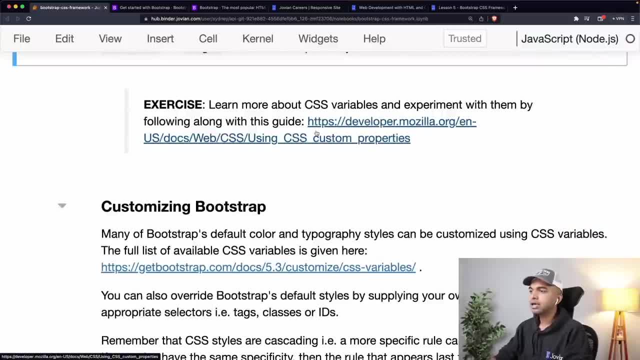 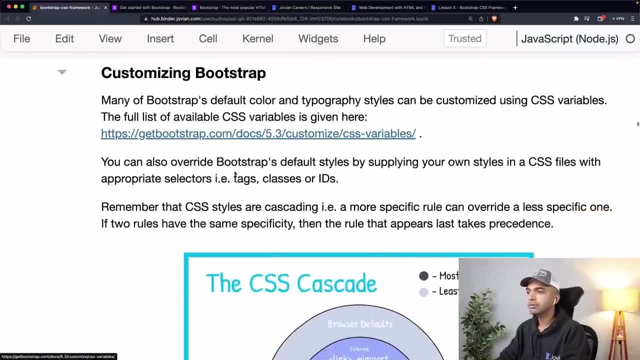 Okay, So you can learn more about CSS variables and experimenting with them. Okay, So you can learn more about CSS variables and experimenting and experiment with them by following this guide on the Mozilla developer network. So I'll let you check it out as well. 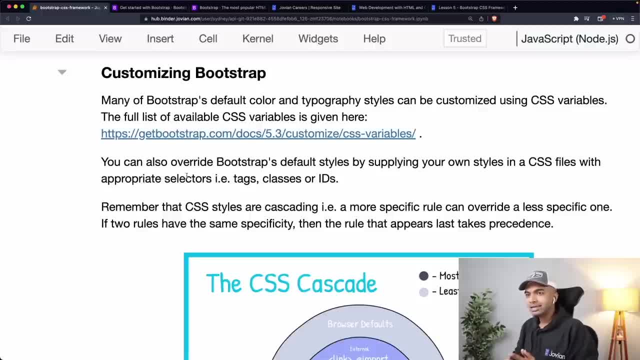 But here's what I want to now tell you. customizing bootstrap is done by changing CSS variable. So many of bootstraps default color and typography settings can be customized using CSS variables, And you can get the full list of CSS variables that have been defined in the bootstrapmincss. 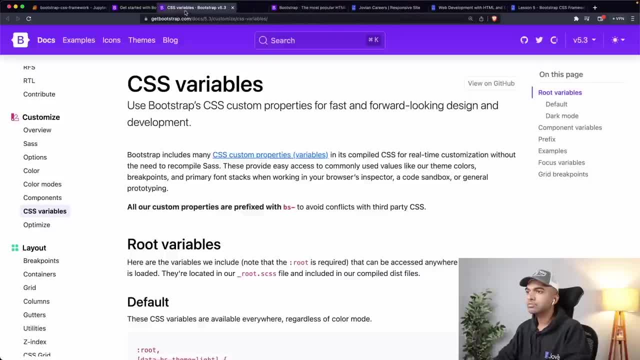 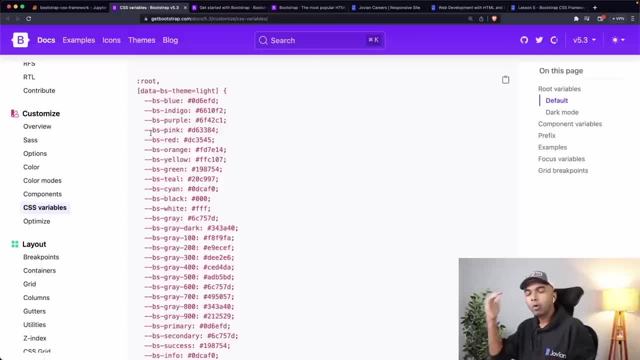 file over here on bootstraps documentation website, So you can see. these are all the variables that have been defined by default, And what you can do is you can now override them in your own style tag or style file, And then what is going to happen is all the bootstrap classes which use these colors are. 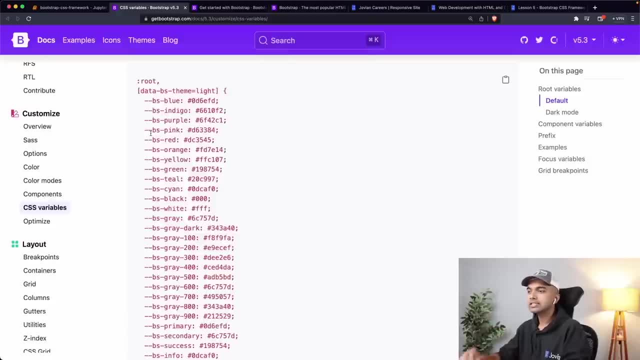 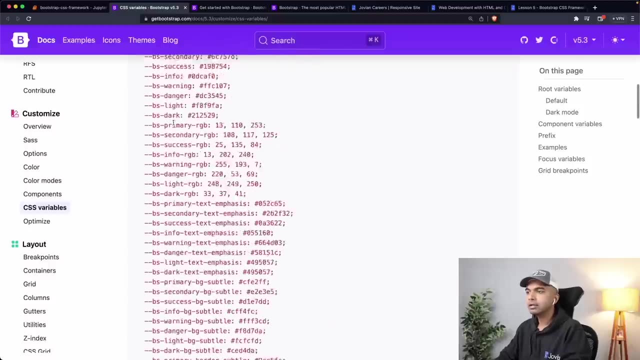 going to pick up the new colors that you've provided or the new fonts or sizes that you've provided. Okay, so I encourage you to check out all the different variables that you can actually modify in in bootstrap. So that's it, Thank you. 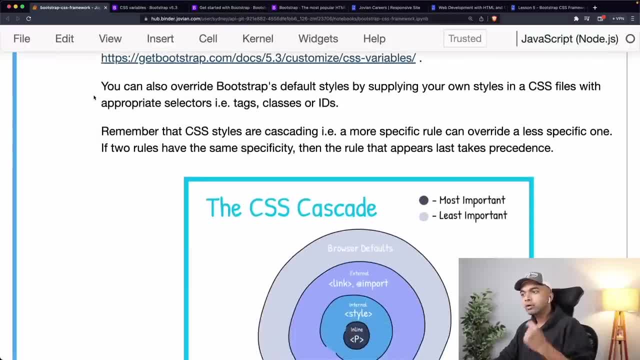 Bye. So that's one way using CSS variables. Another way to bootstrap, to override, bootstrap- default styles is simply by supplying your own styles in a CSS file with appropriate selectors. Let's say, you don't want to change the primary blue color for the entire website, only for 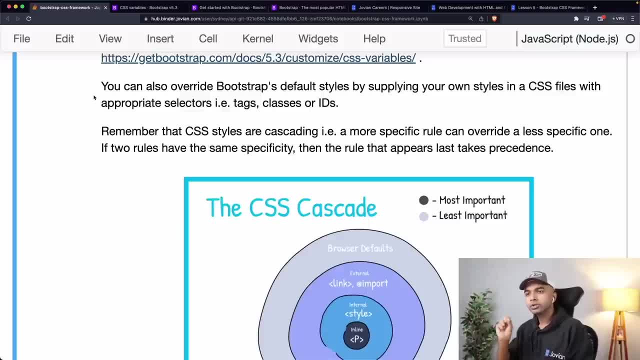 a particular set of buttons in a particular section, you want to change the color. So you can just provide the CSS selector, maybe give it an ID, maybe given a special class, and then in that class you can simply go ahead and apply the changes to that particular button. 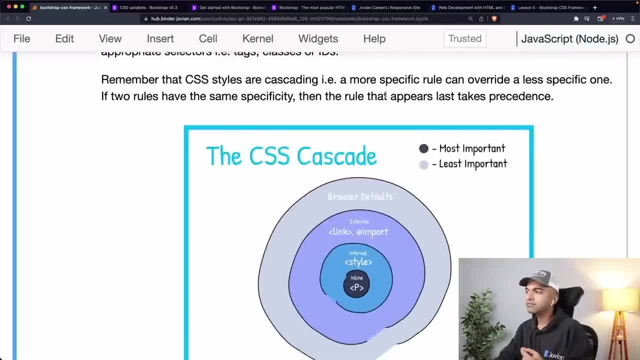 So remember that CSS styles are cascading, which means a more specific rule can override a less specific rule, And if two rules have the if two rules have the same specificity, then the rule that appears last in order takes precedence. okay, and this is something that can be confusing, and 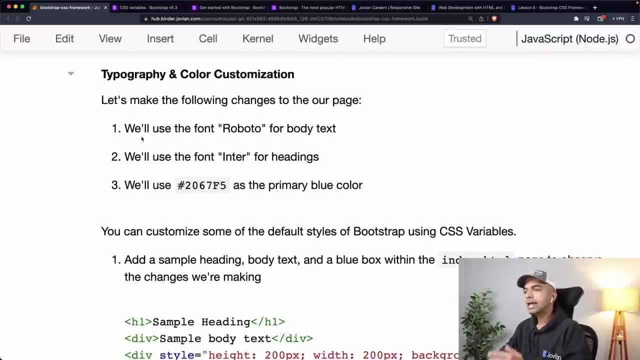 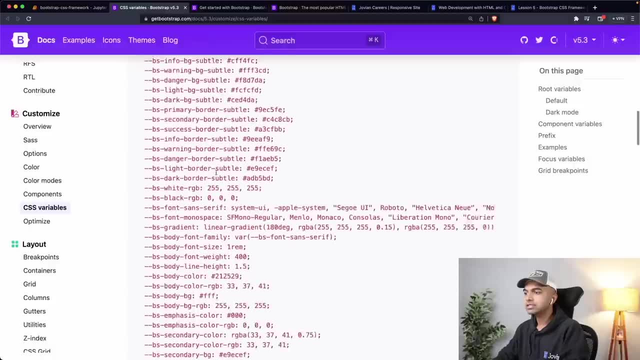 may require some experimentation to understand. So let's make the following changes to our page. We will use a font Roboto for the body text. If you check the CSS variables here, it looks like there is the the font family for the body: BS, body font family. 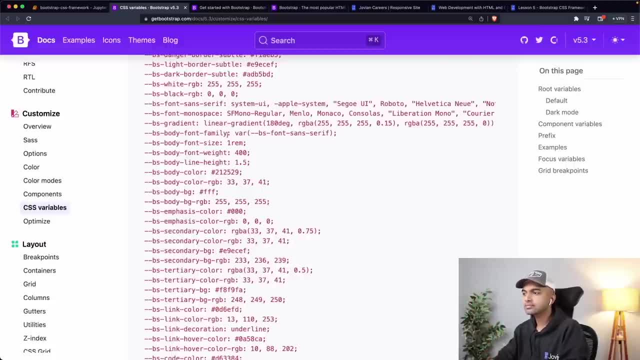 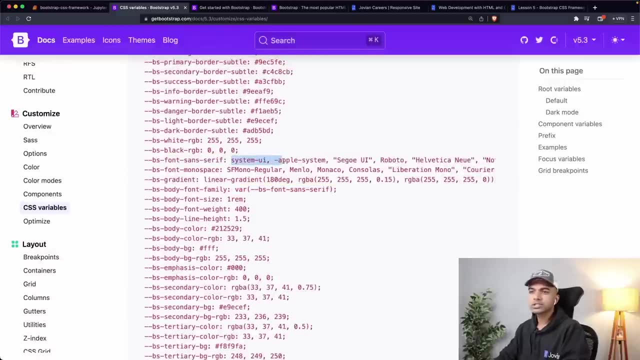 This is what is actually going to be used in the body. If you check the bootstrap CSS file, it itself uses the variable BS font sans serif and looks like BS font sans serif. uses something called system UI, which is simply the default sans serif font in the browser or in the system or in the operating system. 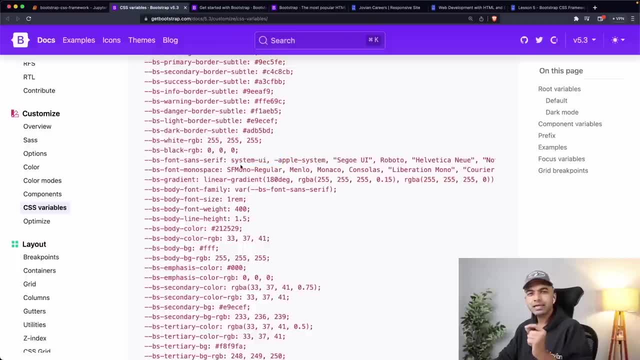 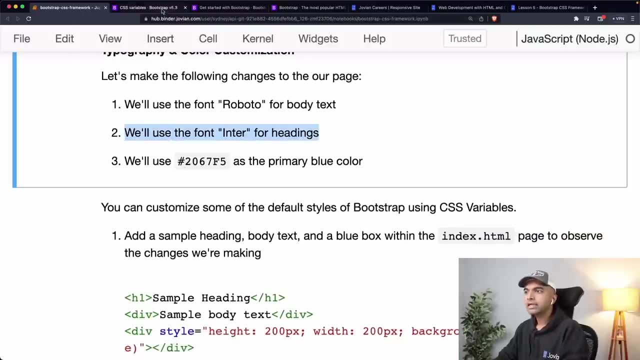 Alright, so we don't want to use this. we want to always set it to Roboto. So that is one change we are going to make. Then we will also use the font inter for headings. Now, if you check here, there is no specific font that has been specified for headings. 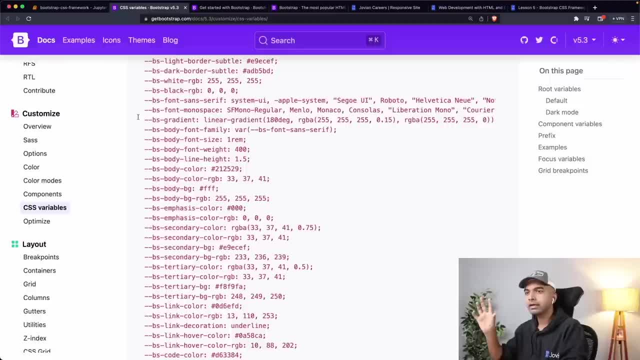 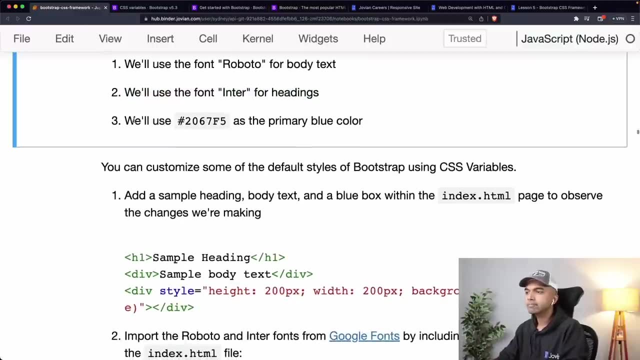 looks like bootstrap by default just uses a single font for the entire page for all kinds of text. So that's where we can probably use some CSS selectors and change the font for headings. And finally, at Jovian we have a specific blue color that we use. 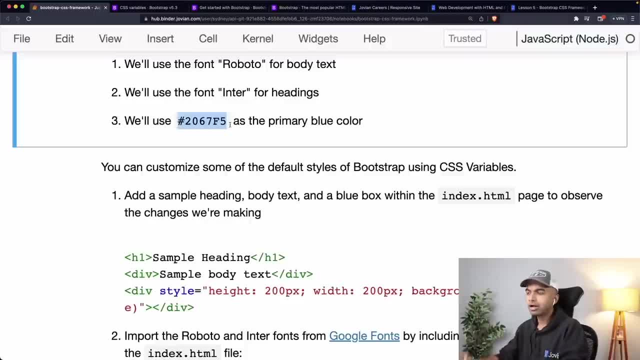 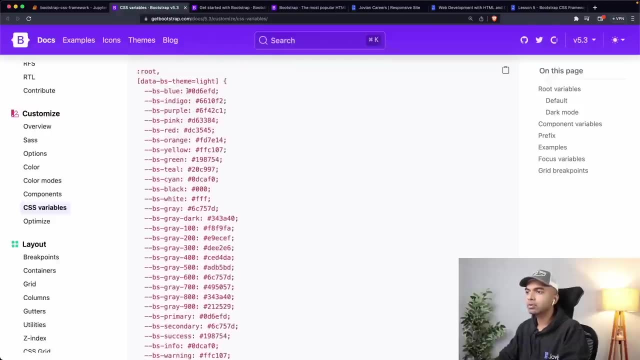 And there are different shades of blue that different companies use. about half the companies on the internet seem to use a blue color for some reason, But we are going to use this 2067 F5 as the primary blue color. You can see here that the primary color that is used for the primary blue and bootstrap. 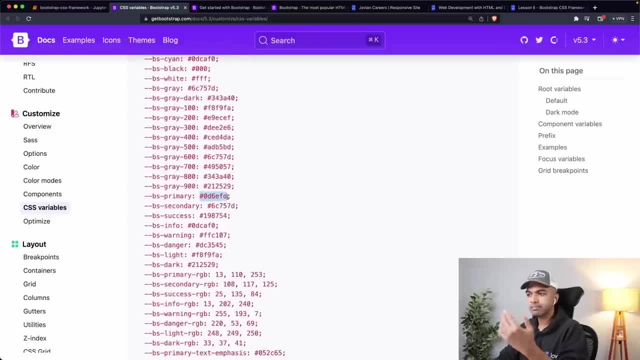 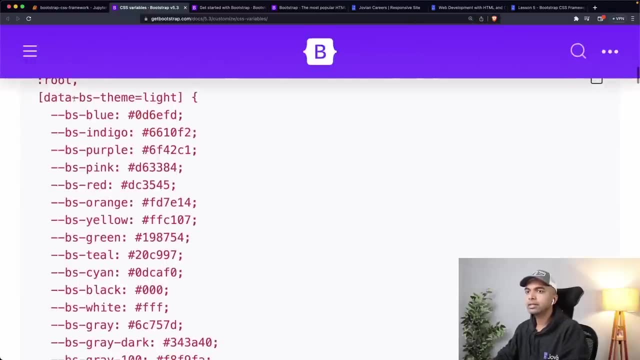 is something else, And there's also this BS primary, which is exactly the same blue that is here at the top. we're going to change both of these, the BS blue- if I zoom in a bit, we're going to change the BS blue color. 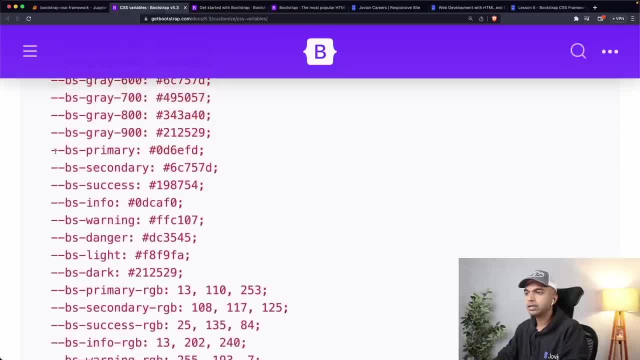 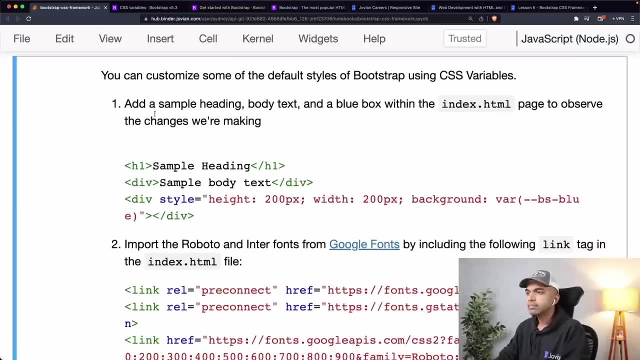 And we are going to change the BS primary color as well to our desired Jovian blue. Okay, So let's start doing this step by step. So first we'll add a sample heading, sample body text and maybe a sample blue box that 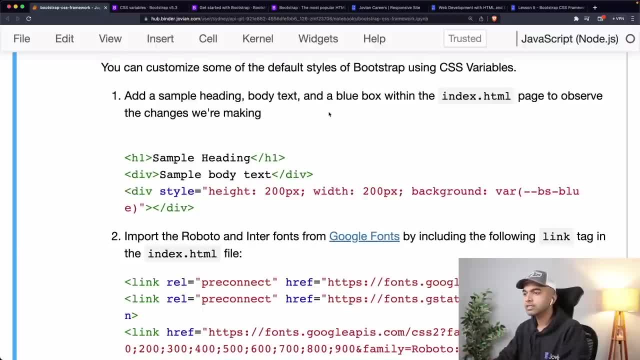 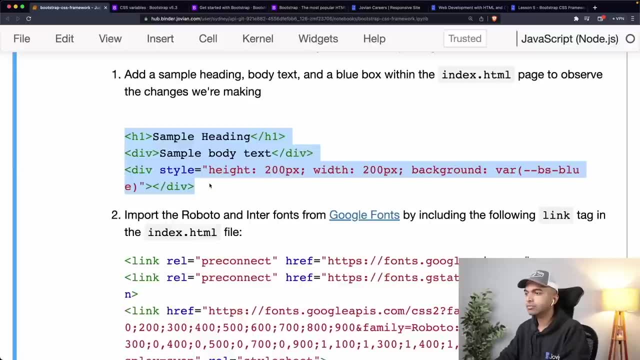 is going to be present in the indexhtml file so that we can actually observe these changes. Let me copy over this H1 tag, this div tag and also this third div or the second div tag, which has a height of 200 pixels and it uses the background var. BS blue. 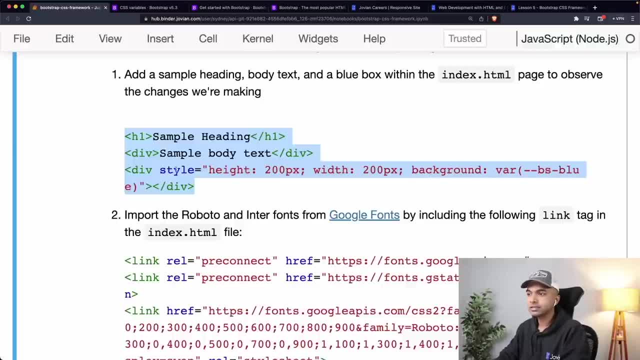 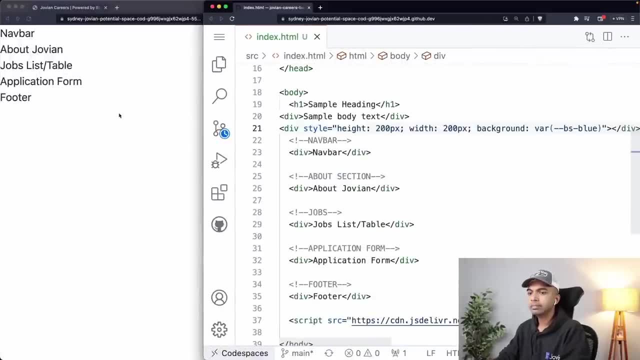 So you can use CSS variables within inline styles as well. So within the actual style attribute. Let's go ahead And let us just put this within the body here and let us save it and let's reload this page, Okay, So now. now you can see we have H1. 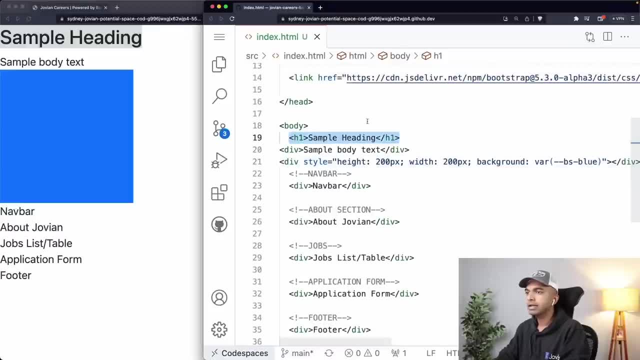 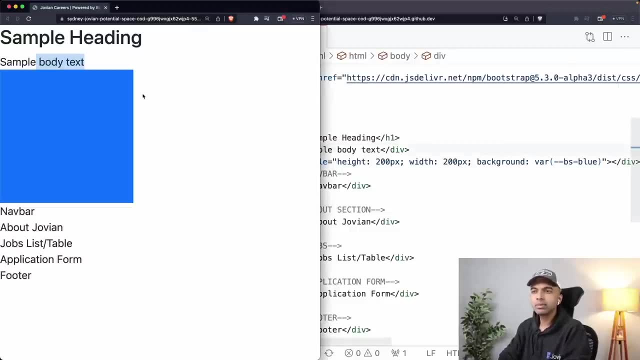 So this is the H1 tag, and the H1 tag has the sample heading, and then we have some sample body text. So I've just created some sample body text And of course I've zoomed in here a bit. That's why it looks big. 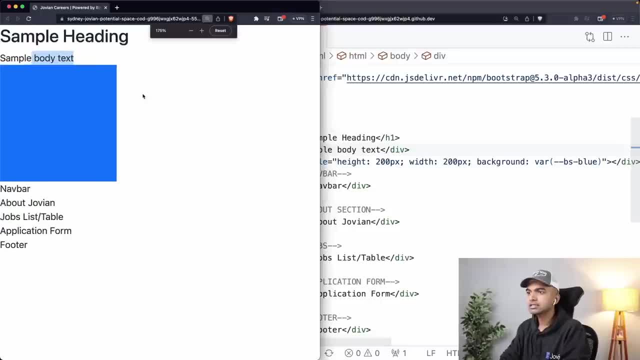 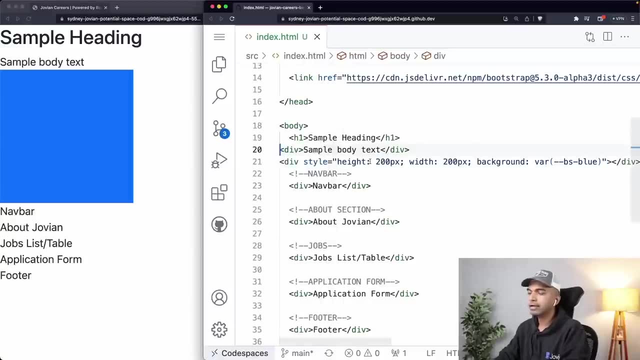 This is the actual size, but let me zoom back in so that you can actually see this properly. And we've created this box here. So this is the sample body, which contains the default blue color of bootstrap as the background. It has a height and width of 200 pixels each. 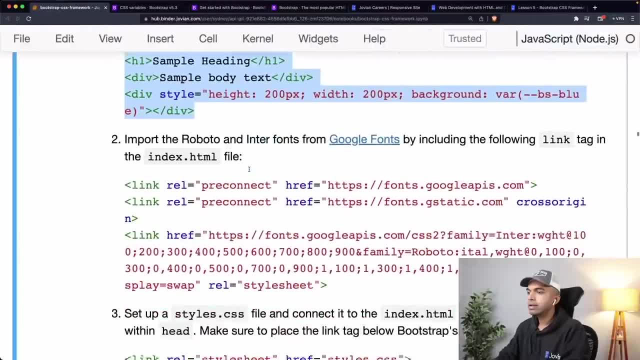 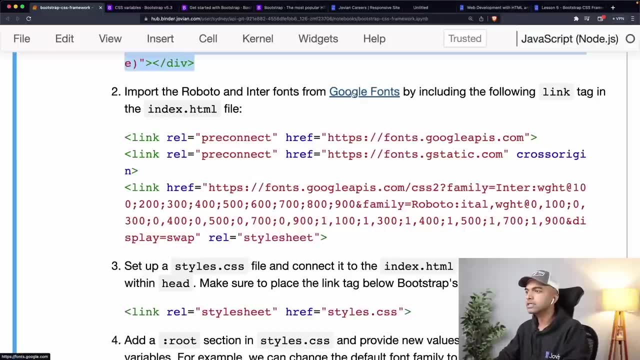 Okay, It's using the bootstrap blue as the color. Next, we can now first to change any fonts. we have to first import fonts from Google fonts. So you can always go into Google fonts and let's say there are a couple of fonts that 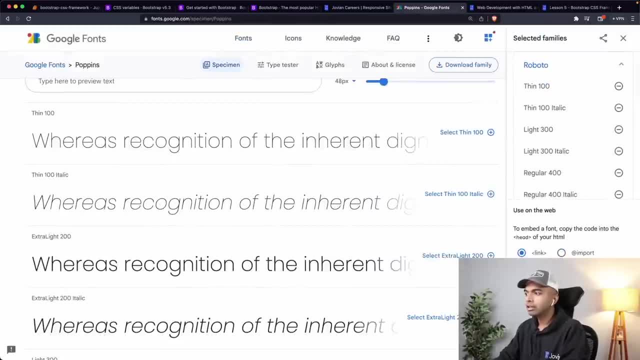 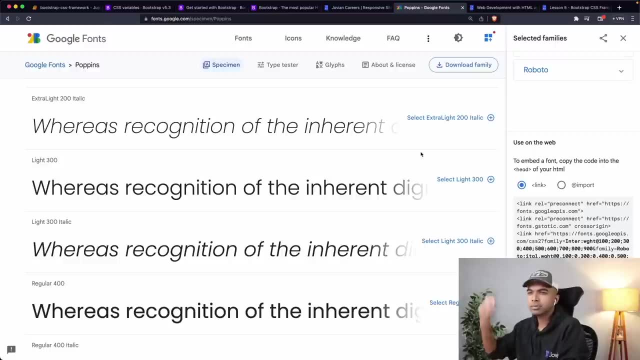 you need to use. You can go into that particular font, You can add all the styles that you need And once you've added all the styles- which I've done here for inter and robot, Okay, Okay. So you should be able to copy over pretty much all the styles because you might need. 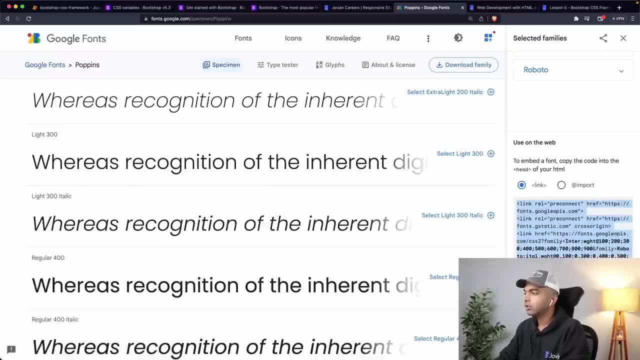 you don't know which one you might need, Then you can come in here and you can actually go ahead and copy a link tag. So if I zoom, if I scroll up here, you can see that there is this link tag that can be. 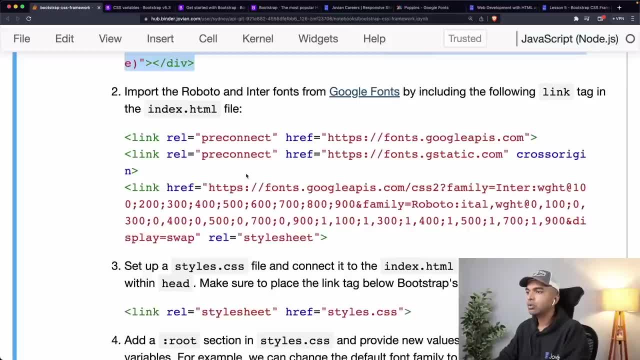 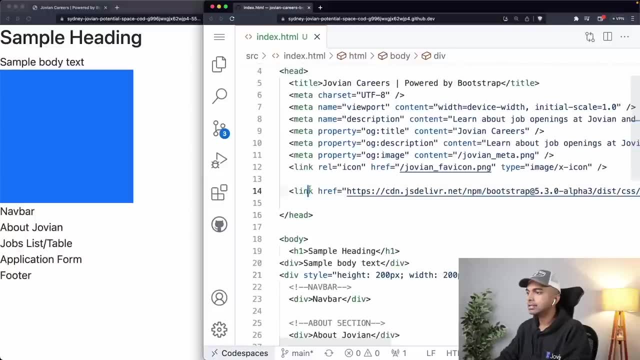 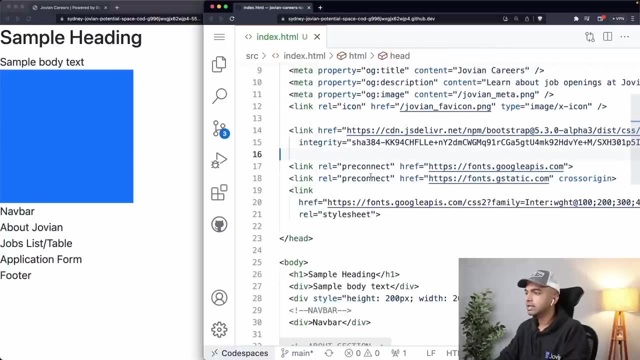 copied And that link tag has to be added into our index or HTML file to load these fonts from Google fonts onto the page. Okay, So I'm just going to add this link tag right below my bootstrap link tag, Okay. Okay, So I'm just going to add the document once again as well. 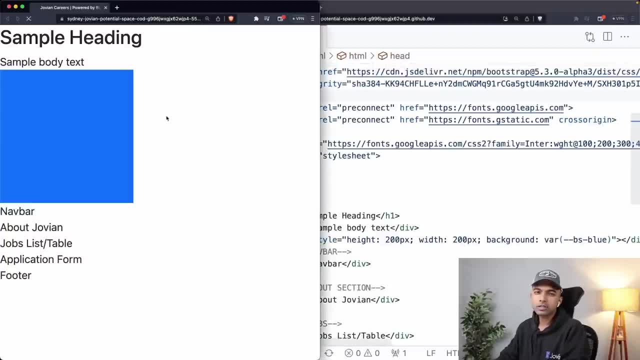 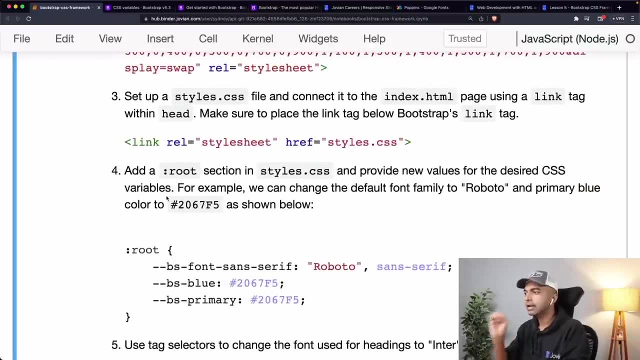 Perfect. So now we've included some fonts, but of course, no change has been made yet because we've not actually used those fonts. next, Let us set up a styles or CSS file and connect it to index or HTML using a link tag within the head. 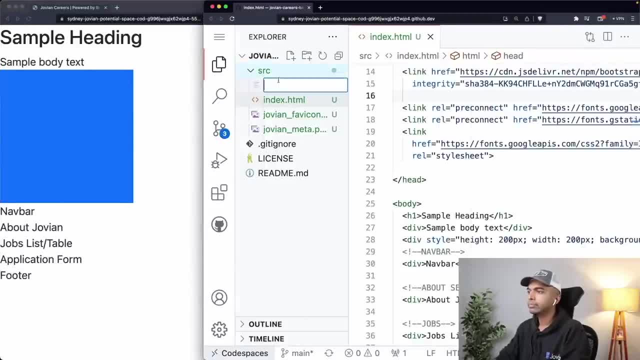 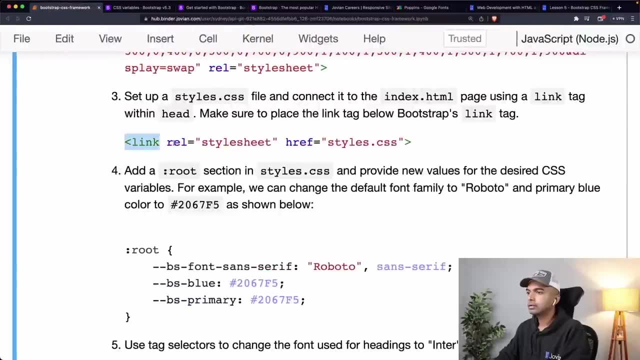 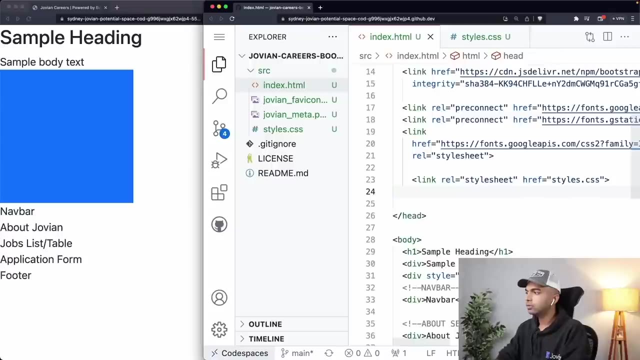 So I'm going to come back in here. I'm going to create a file stylescss and I am going to link it using a link tag. So link rel equals style sheet, href equals stylescss. So I'm just going to put that into stylescss, into the index or HTML file. 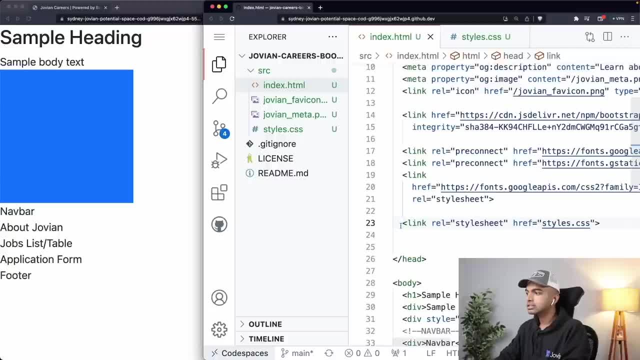 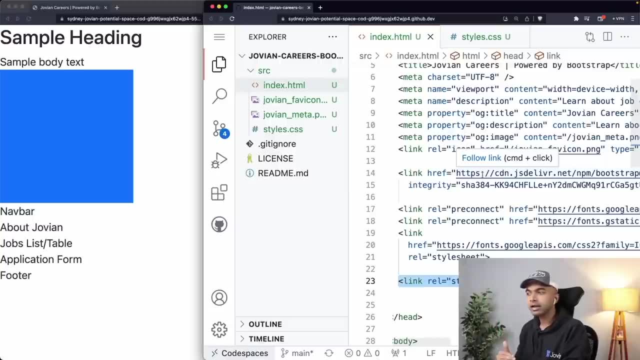 Now, one important thing you should keep in mind here is you have to put this- your custom styles- below the bootstrap styles, because that is the order in which the CSS variables will be read. So if you put it above, what's going to happen is: first your CSS variables will be read and 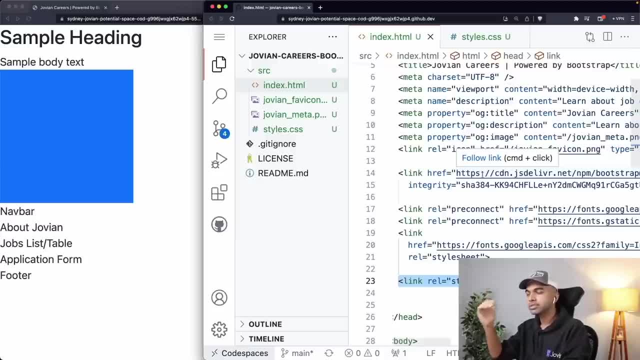 then the bootstrap CSS variables will get read and those bootstrap CSS variables will override your values. But you want to do the opposite, Okay, So you want to take the bootstrap CSS variables and you want to override them, And then all the classes that are present in the bootstrap CSS file will automatically. 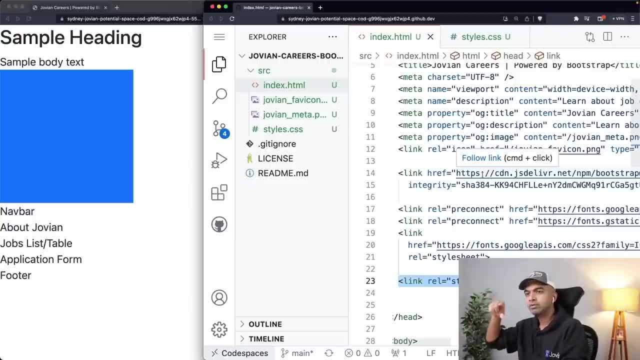 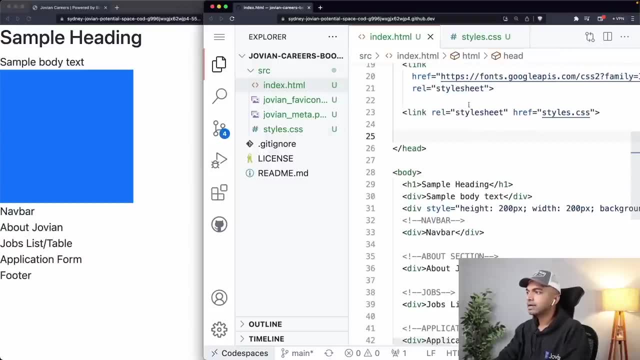 pick up the overridden value. So that is the interesting way in which you can go back and you can change some of the styles in in bootstrap. Okay, Alright, so now we have the stylescss file. still, there is no change. that has happened. 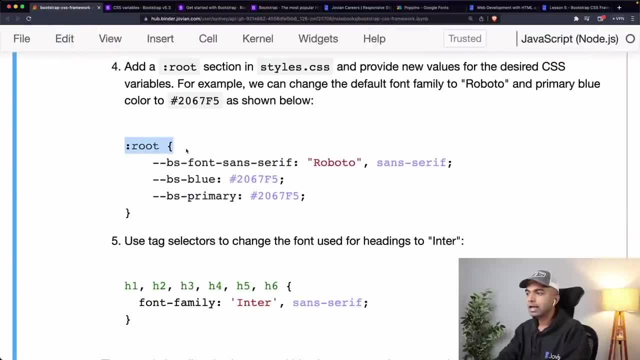 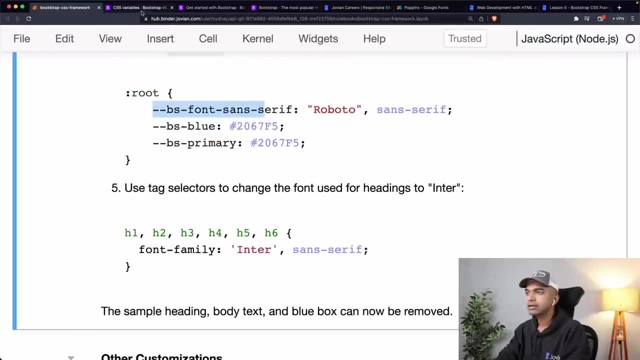 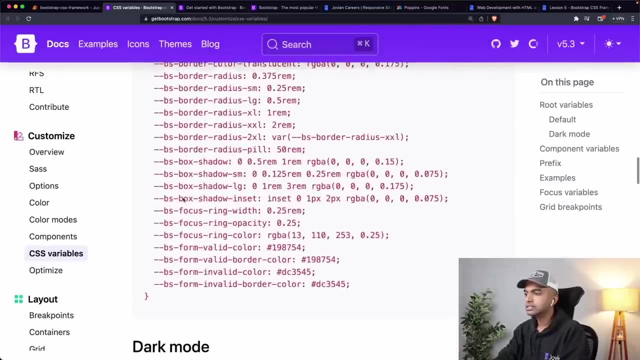 Now let us start by first adding this root tag and then changing a couple of or three properties. So we're going to change the variable BS font sans serif. You can see here that there is this BS. there is this BS font sans serif. 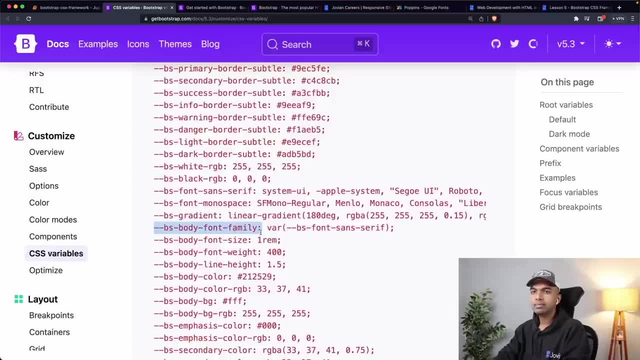 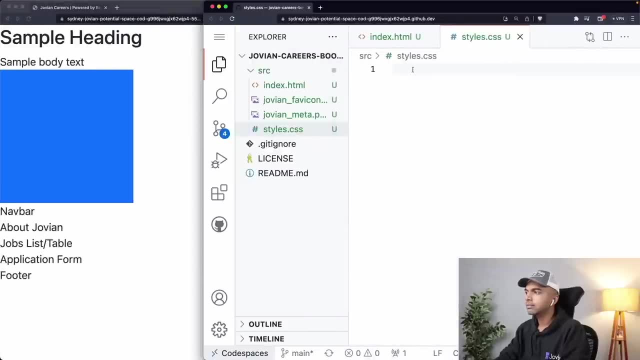 This is what is actually going to be used as the body font family. So the body font family variable gets used in the body, if you study the bootstrap structure. So I'm just going to come in here and I'm going to create the root tag. 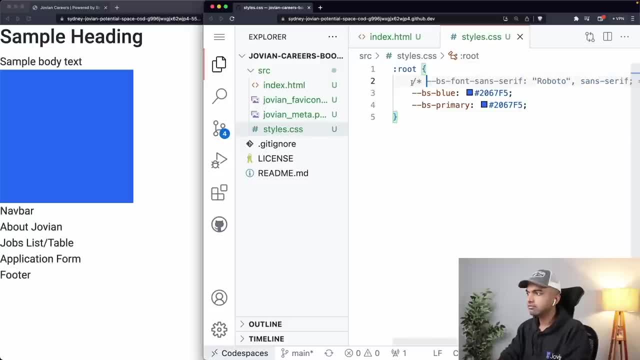 And you can see as soon as I pasted it, a bunch of things have changed And we can disable these And we can observe the changes one by one. First, let us keep an eye on the text over here As soon as I enable this. you can see that there has been a slight change in the text. 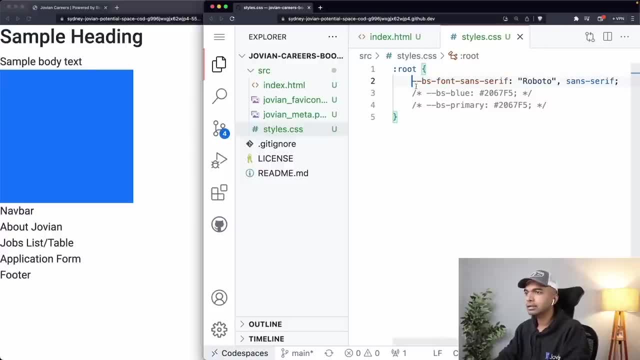 It's very, it's very minute, But if you just look at it carefully, you see this is different And this is different, right? So these are minor changes in the font, But you want to get the company font, the font that your company uses. 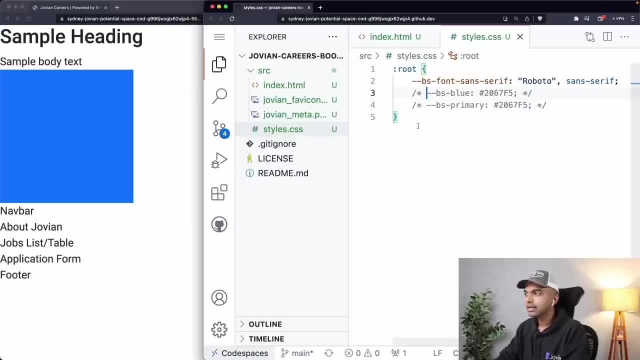 That's why this is important. Let's then change this blue color as well. Again, it's going to be very subtle. Yeah, so looks like there's a minor change here in the blue. you may not even be able to detect it. 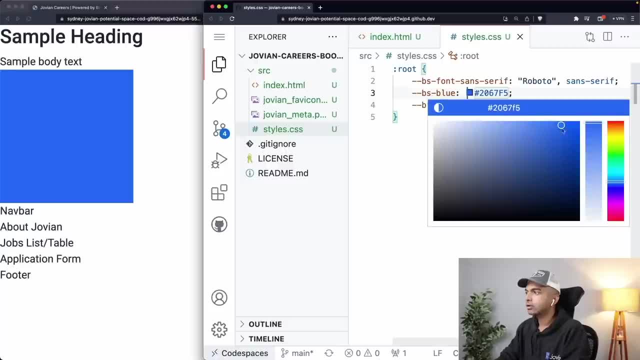 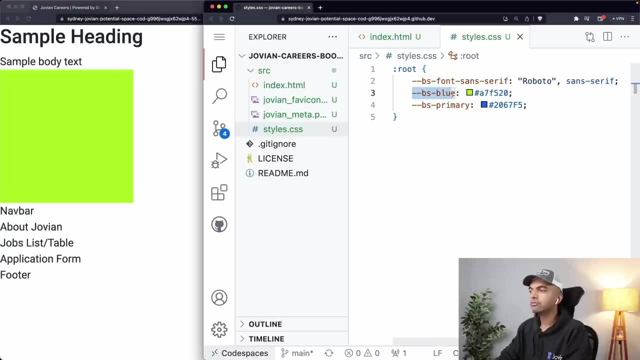 But I can always go in here And just for the sake of testing, I can go in and maybe make this a green color And you can see that now the color changes to green, right? So whatever value you set for the BS blue CSS variable, that is going to override the 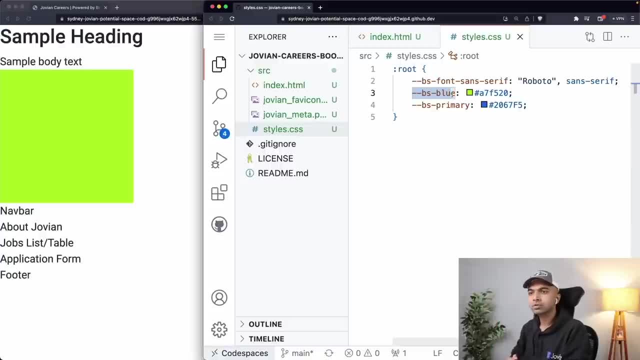 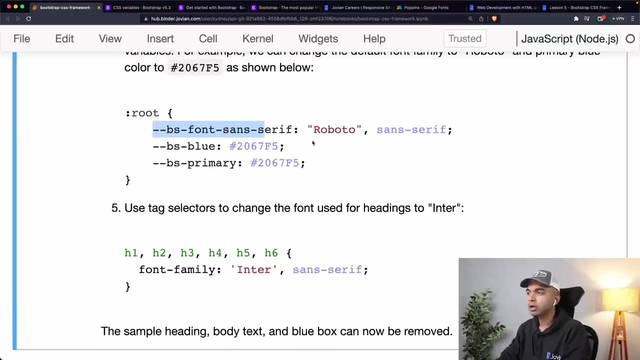 default value in bootstrap And that is then going to be used within all the classes, within wherever you want to use This color. Okay, so I'm going to reset it back to the color that we had for Jovian And just like that. we have modified a few basic styles. we modified the body font, family. 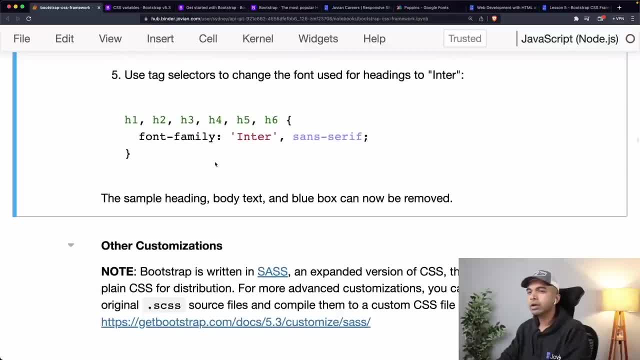 and we've modified the blue and primary colors to our desired color. Of course, we also want to use the inter font for headings, So that is something that we can simply do by adding these selectors, h1 to h6. And we can simply set their font family to enter with a fallback to sans serif. 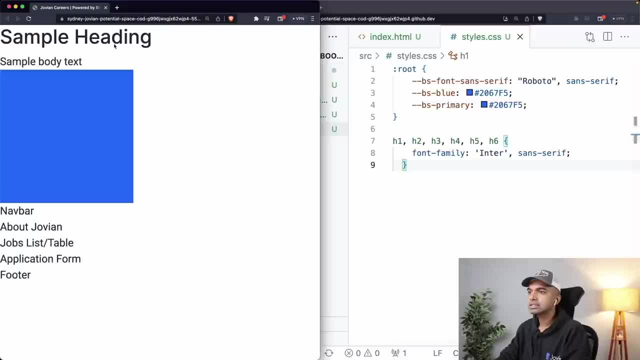 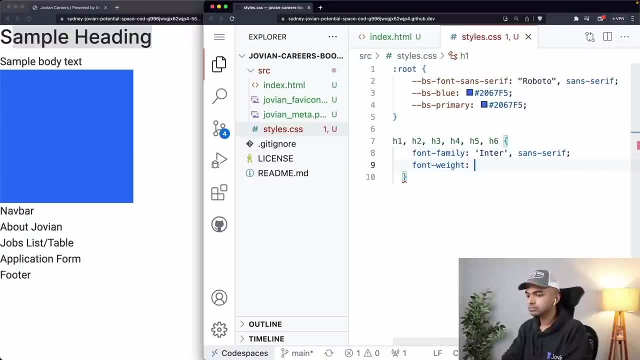 If the font could not be loaded. So let me come in here And you can see that there is a slight change here to the heading, And I can even come in here and maybe not check out the font to wait six and set that to 600. 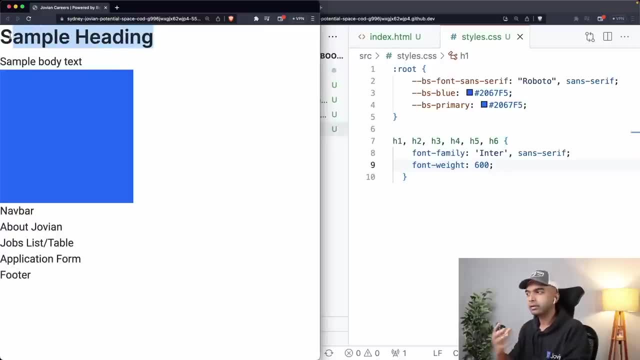 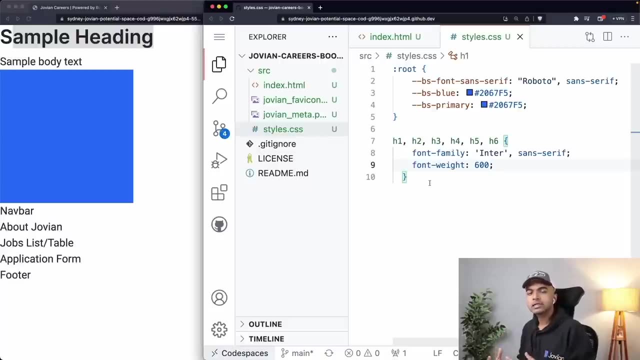 You can see now my fonts on my headings are a bit thicker, So remember that. if just because you've used bootstrap does not mean you can not use your own CSS styles, you can customize pretty much everything in bootstrap, And the simplest way to do it is often to just add a class. 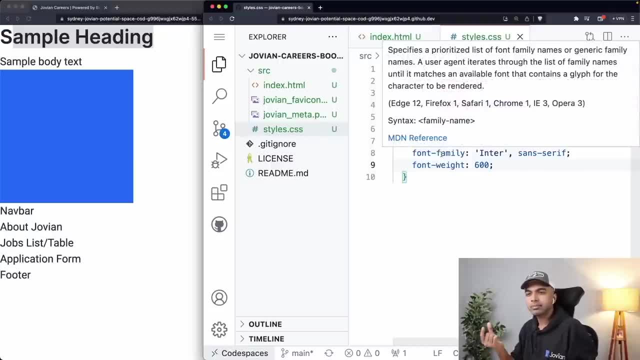 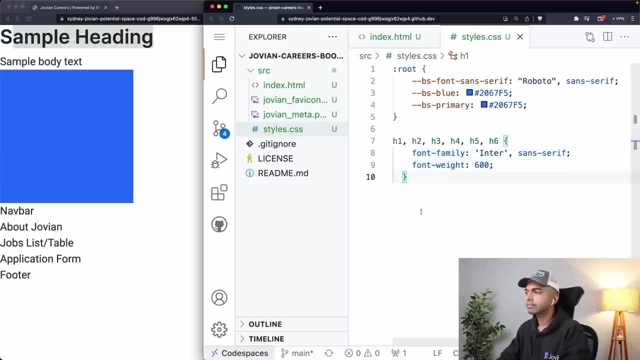 Let's say this is a class. If there's a particular button you want to customize, just add a class to that button and simply go into your CSS file and then apply the styles to that particular button or div or whatever. it is Okay. 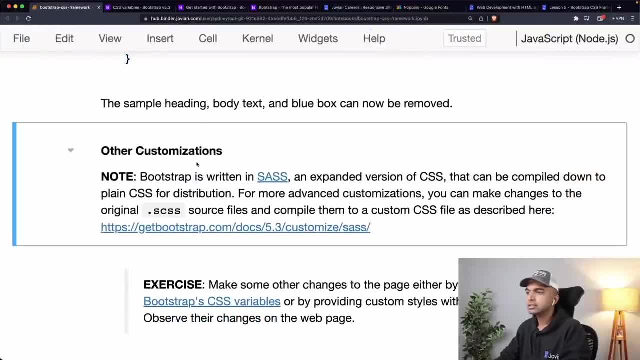 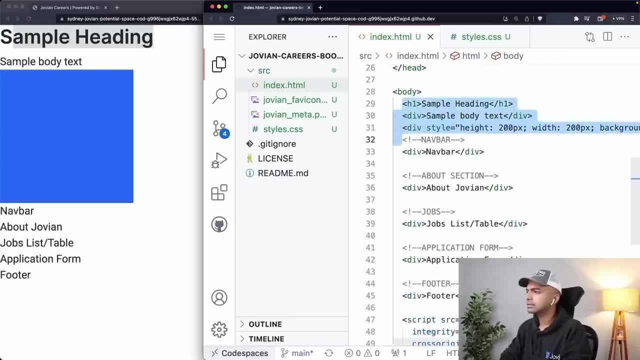 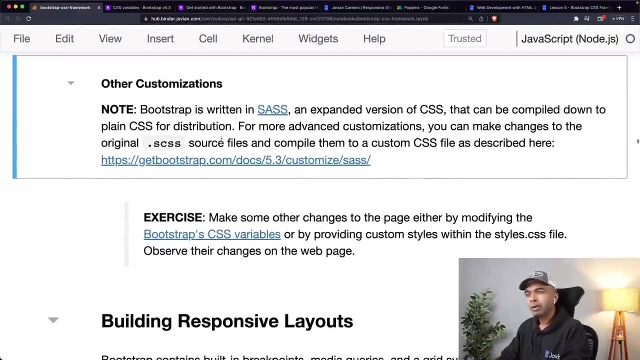 And with that we have performed a bunch of customizations does, and we can now get rid of the sample heading, sample body text and sample div that we had And we can proceed with the rest of our website. Now I want to point out that 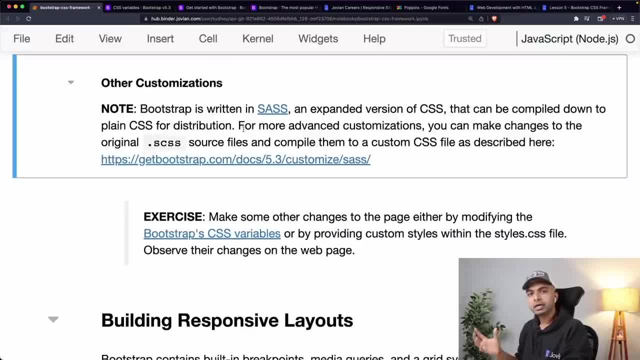 There's actually a much more, much deeper customization that you can do at a very specific component level within bootstrap, and bootstrap is written using this language called SAS, which is essentially an extension of, or an expanded version of, CSS that can then be compiled down to plain CSS for distribution. 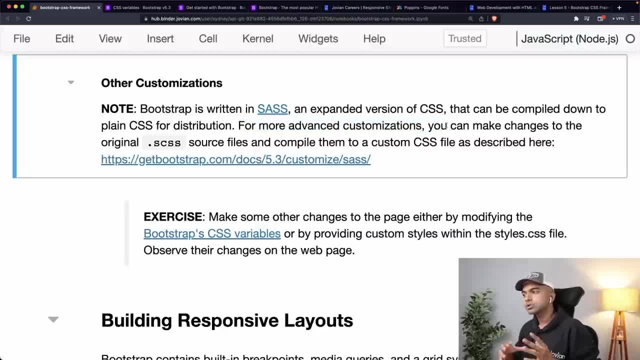 And for more advanced customizations, you can actually go into bootstrap source code. You can make changes to the original SCSS files- which is what bootstrap is written in- that this is the format of the file- and then compile them down to your own CSS file. 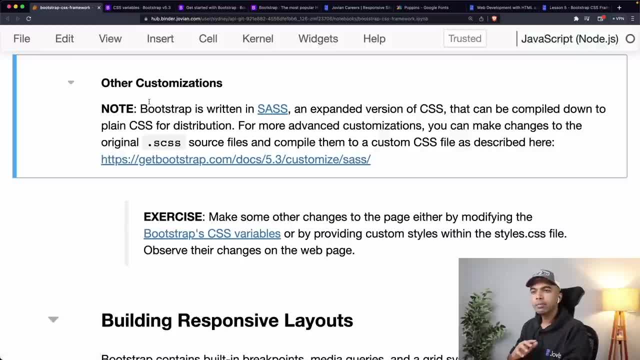 And all of that is described on the bootstrap documentation website. Okay, Most of the time you will not need to do this, but in some certain cases where you cannot figure out a way to do it by using CSS variables or using custom classes- you can go ahead. 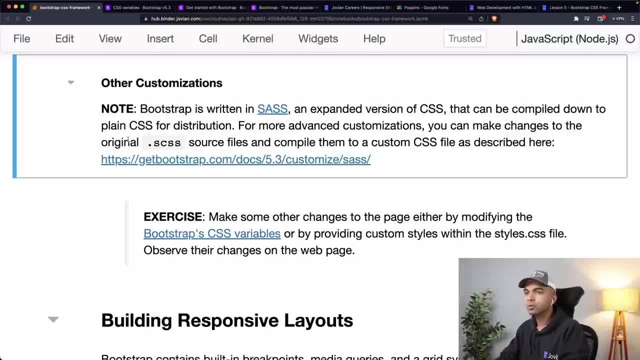 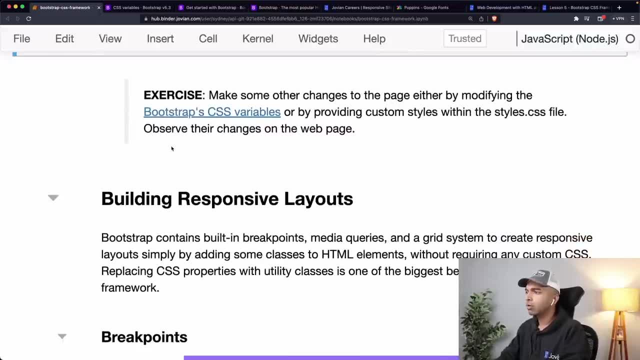 and simply edit the SCSS files and generate a new CSS file for your project. Okay, So as an exercise, I would encourage you to Maybe make some more changes to the page, either by modifying bootstrap CSS variables or by providing custom styles within the stylescss file, and observe that changes on the webpage. 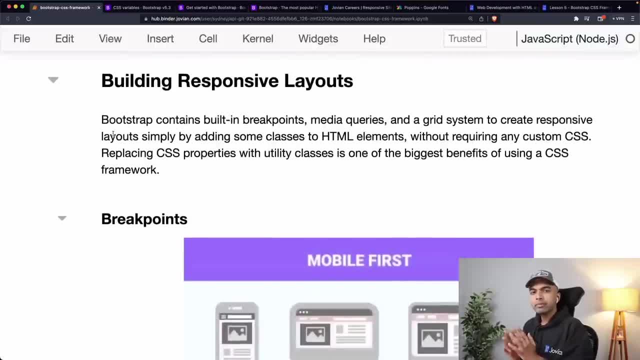 Now let's talk about how we can build responsive layouts. So bootstrap contains built in breakpoints, media queries and a grid system to create responsive layouts simply by adding some classes to HTML elements without requiring any custom CSS. And this is one of the nicest things about using bootstrap: that you don't have to write. 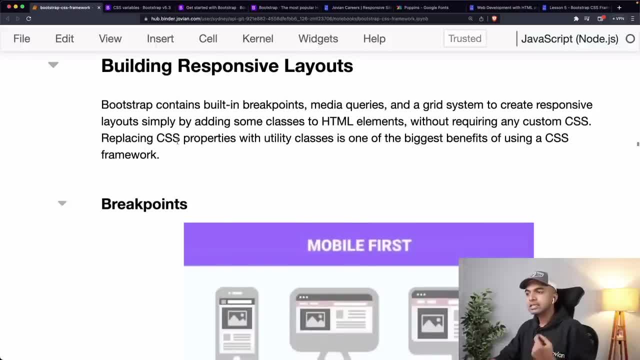 breakpoints and media queries yourself. replacing CSS properties with utility classes is one of the biggest benefits that you can get from a CSS framework, And we will explore multiple CSS frameworks over the course of this program, this course and future courses, but all of them will have this common pattern that they're going to 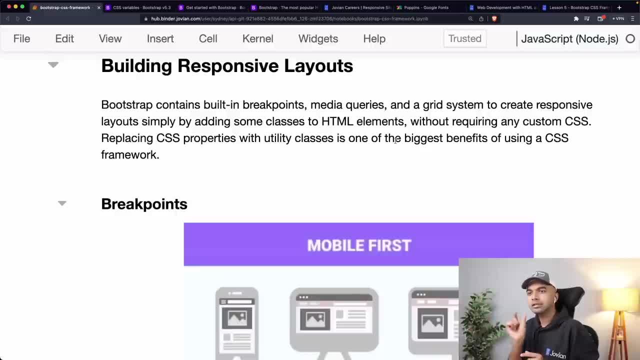 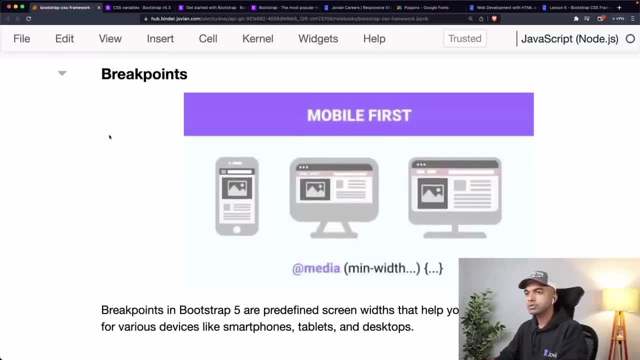 take away some CSS that you had to earlier write manually and just turn them into simple classes that you can include within your HTML file. So first let's understand the built in breakpoints and bootstraps. So in bootstrap, because it's still useful for us to know this. 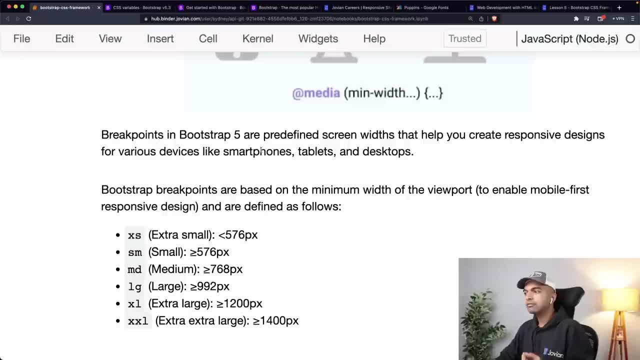 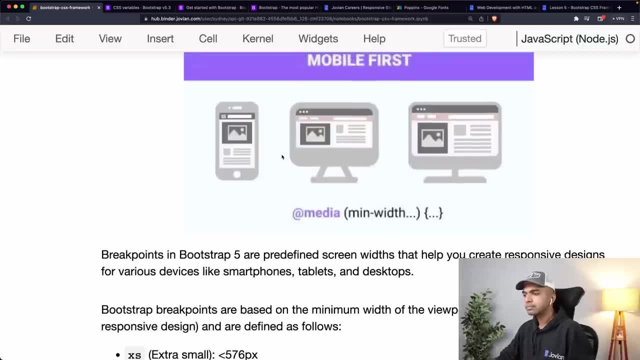 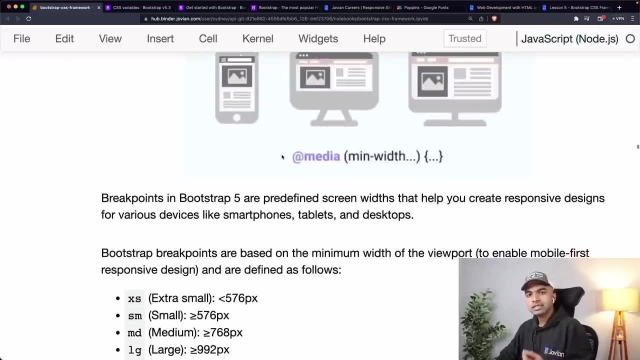 So breakpoints and bootstraps are in. bootstrap are predefined screen widths that help you create responsive designs for various devices like smartphones, tablets and desktops, And bootstrap uses a mobile first approach, which means that the boots- which means that the styles that you supply for the smallest breakpoint- will automatically follow through. 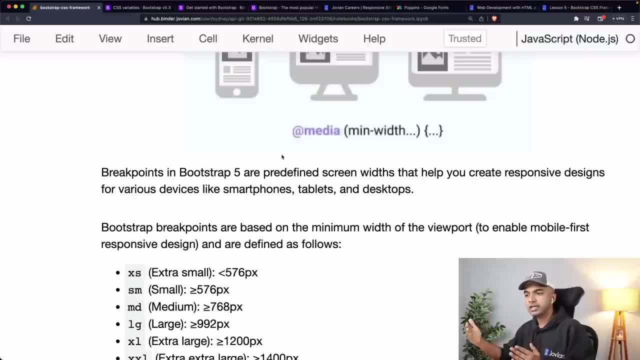 or get applied to bigger breakpoints until you choose to change them. So that is where you should always first design the mobile version of your site, make sure that it looks good on mobile And by default, all those styles will carry over into the bigger layouts as well. 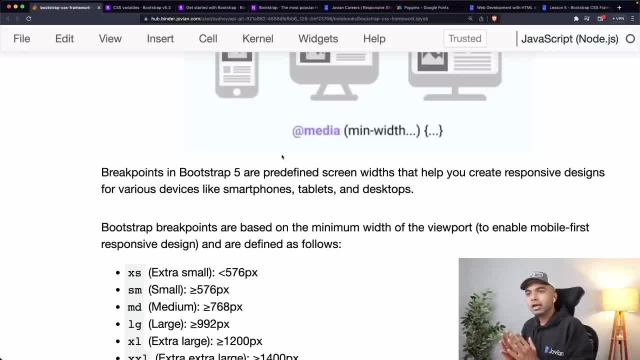 And then you can specify some custom styles when you get to a tablet layout and just make the required changes that you need, And then you can again go to a desktop layout and specify some more changes. So that is called mobile first responsive design with incremental adaptation to increasing. 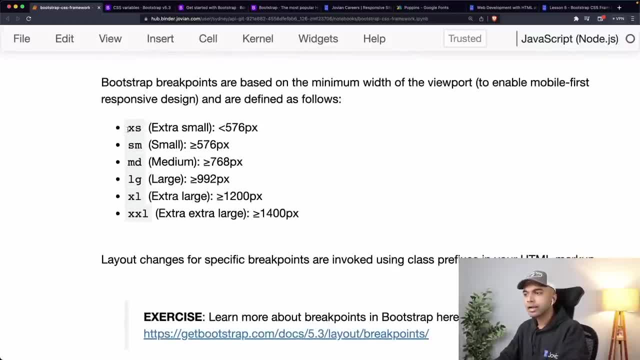 screen size. So by default, the styles that you supply to bootstrap, they get applied on excess screens, which is screen smaller than 576.. But of course they also carry over to bigger screens. then, if you can, if you supply some, 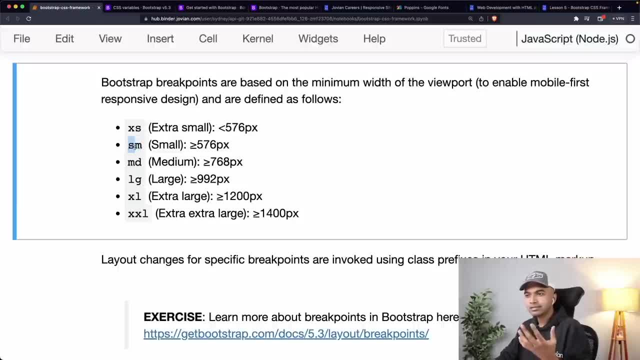 style for the SM screen and we'll see where this SM word actually gets applied- then that is going to only apply to screens that are bigger than 576 pixels. Then if you want to apply some styles for bigger or browsers with a bigger size, then 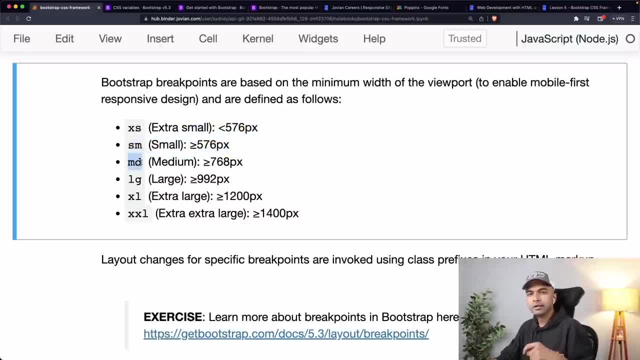 if you want to apply some styles with a bigger width, with width greater than 768 pixels, you then use the MD And then, similarly, there's a breakpoint for LG, Excel and XSL. Okay, so the way you create layout changes or specific breakpoints is not by writing. 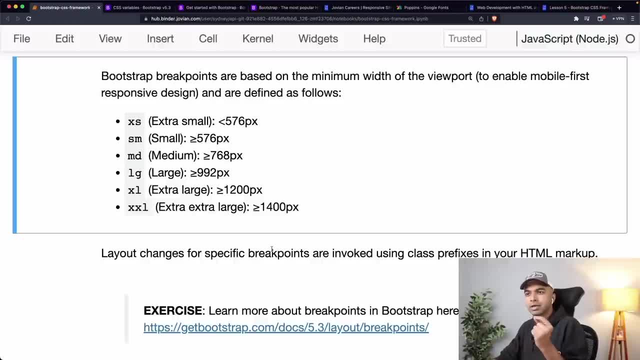 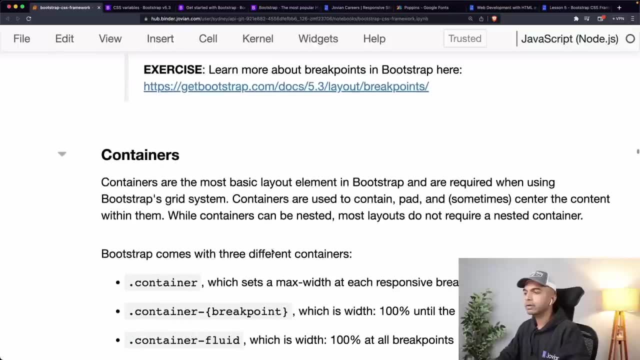 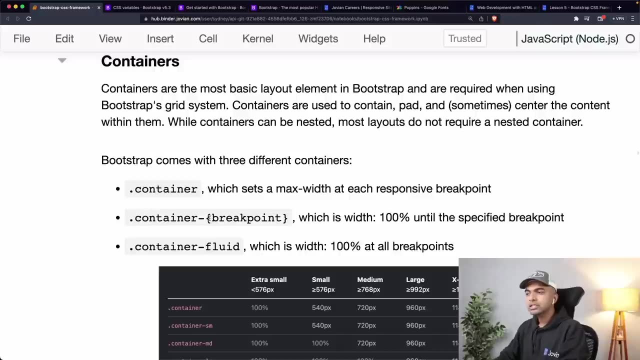 media queries, but by simply using certain class prefixes in your HTML markup, And don't worry if that doesn't make sense right now, because we're going to see an example of that very shortly. So the first key component That we are going to use from bootstrap, or the first key layout element, is containers. 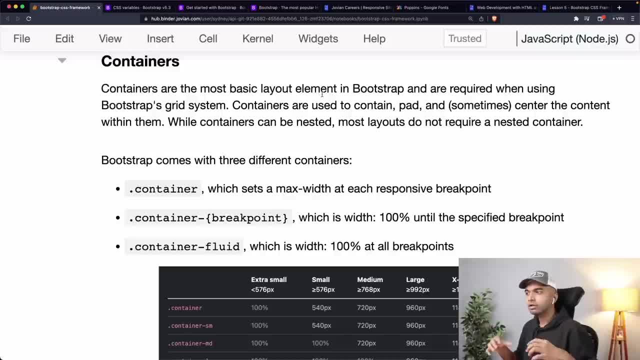 And whenever you want to use some kind of a responsive layout, whenever you want to do something interesting with bootstrap, where the layout changes across different widths, you have to first create a container. okay, And the way you create a container is by simply adding the class container to a div. 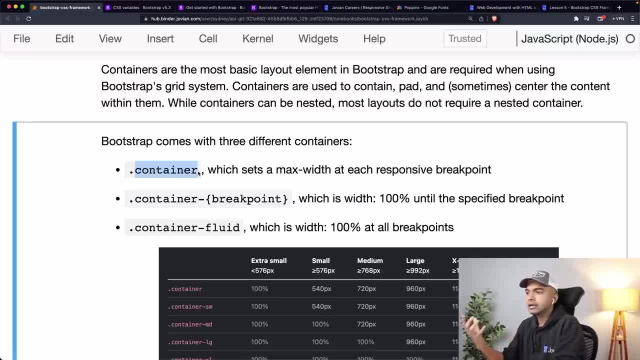 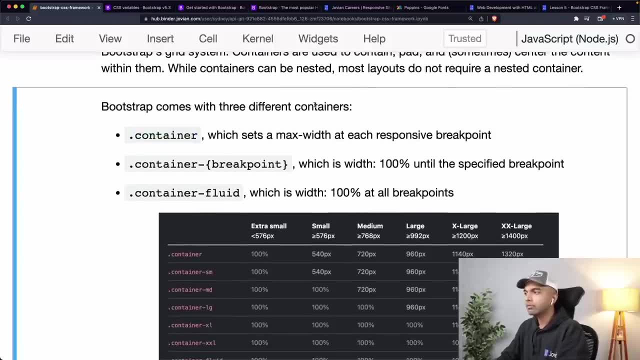 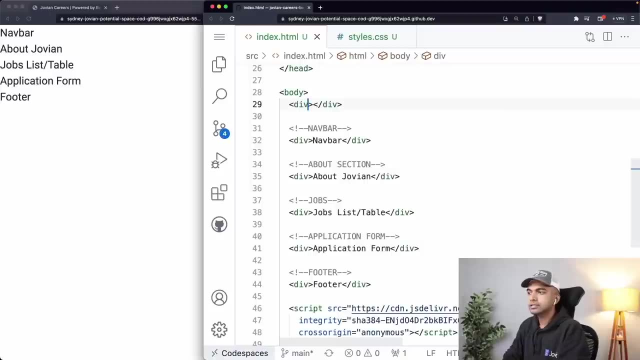 That's it. So you create a container by creating a div and giving it the class container. Now bootstrap comes with three different containers, Or three different types of containers, And we'll take a look at them one by one. So the simplest container that you can create in bootstrap is just by creating this div. 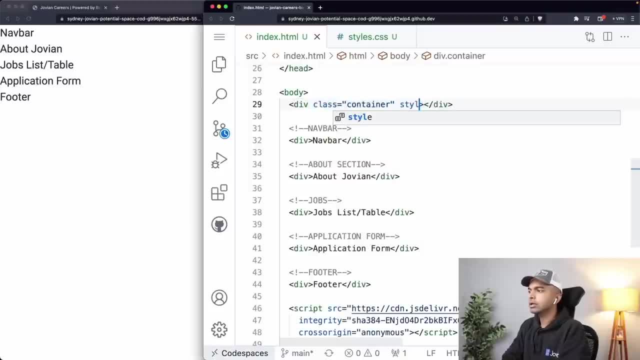 and giving it the class container. okay, I'm also going to give it a height and width. So I'm just going to give it maybe a width of 200px, height of 200px. Actually, let me just give it a height, not a width right now, because the width is a. 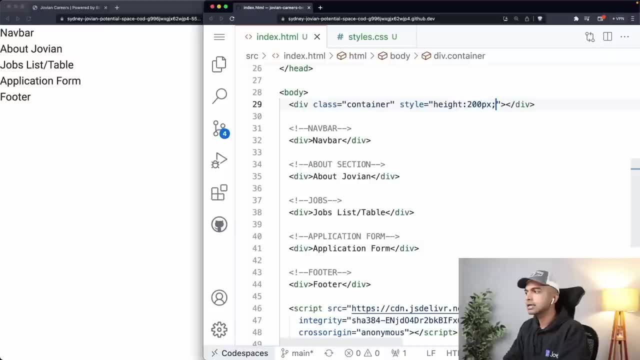 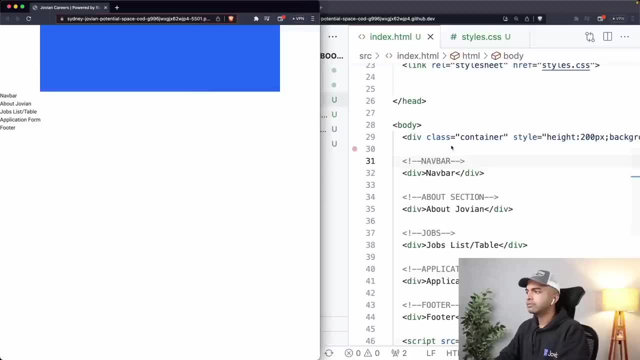 going to be set automatically. So I'm going to give it a height of 200px And I'm going to give it a background of: let's use the blue, BS blue. Now we have this container, we have just created a div with a class container and you've given 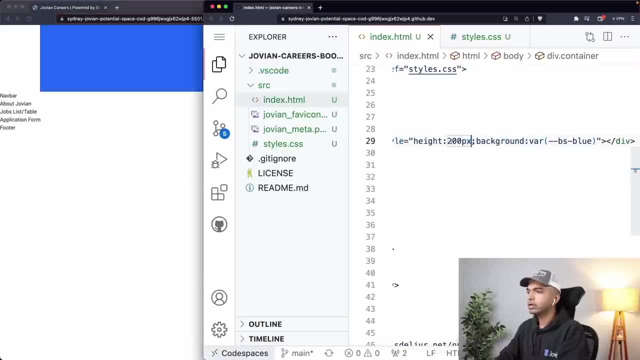 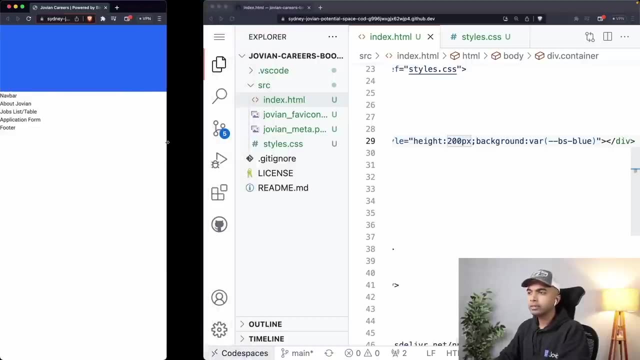 it a height of 200 pixels and a background of blue, And you can see here that this container has this property, that it is always centered on the page And you can see when the when the page is really small. maybe let's use browser tools. 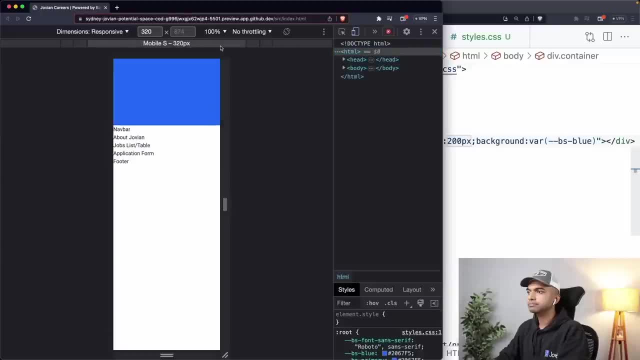 to see this. It's going to be slightly easier to do it this way. Yeah, you can see that the when the page is very small, it takes up the full width of the page, But as we start increasing as soon as we cross the excess boundary. okay, now looks. 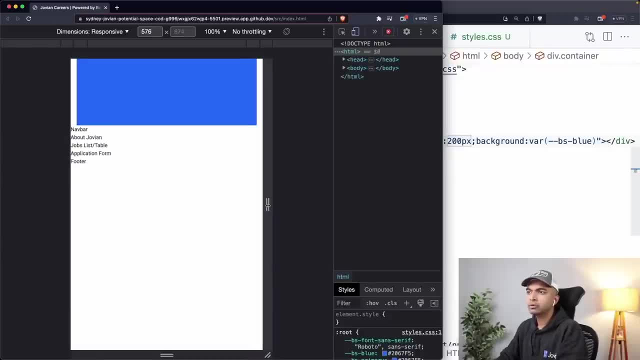 like up to 500 and, okay, up to 576 pixels. it takes up the full width and then its width reduces and it just remains centered on the page And then we hit the next breakpoint, which would be about 768 at 768, it becomes a little. 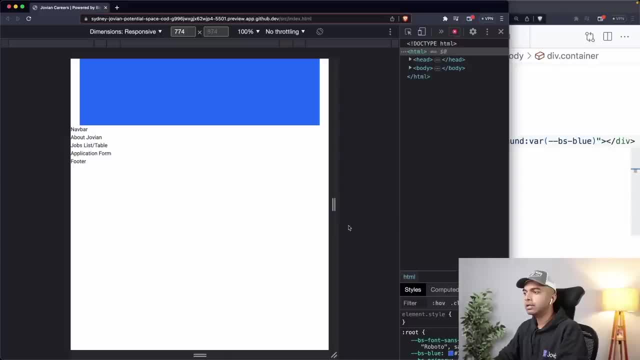 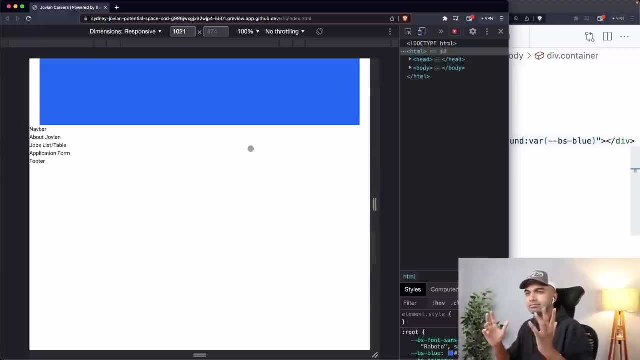 bigger, but it still remains centered on the page, it still does not take up the entire page. And then, as we keep going, we had the next breakpoint. And then, when we hit the next breakpoint, at around 996 pixels or so, it once again expands. 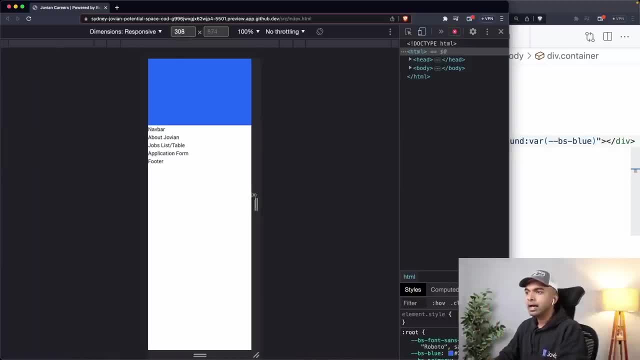 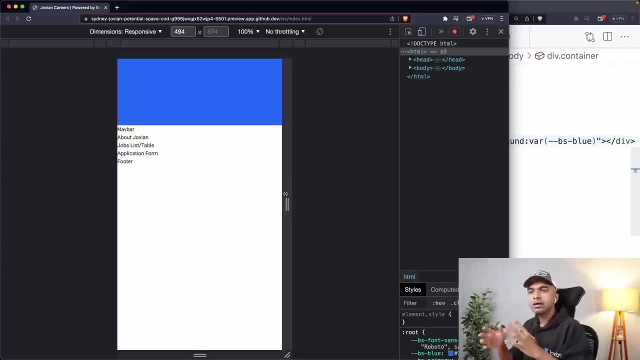 and it remains centered in the page, and so on. Okay, so this is what happens when remember we were doing all this business of setting a cut, of first creating a div and then centering it using margin zero auto by adding left and right equal margin. 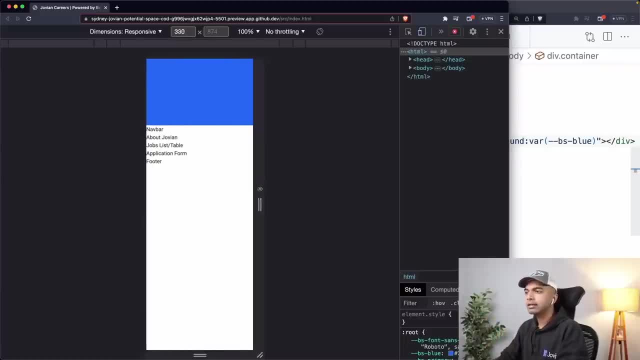 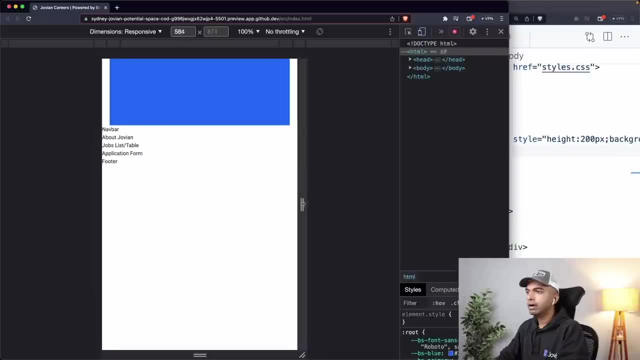 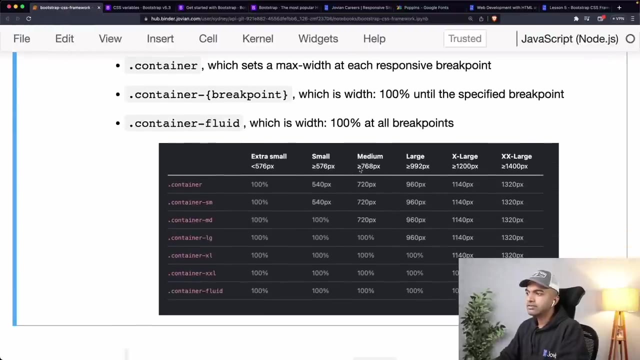 And, at various breakpoints, Adding various widths. well, bootstrap has already done that for us And you can simply add the class container. And when you add the class container till about 768 pixels or so, so till about the, let's see what this means. yeah, till about 768 pixels. it's going to occupy the full. 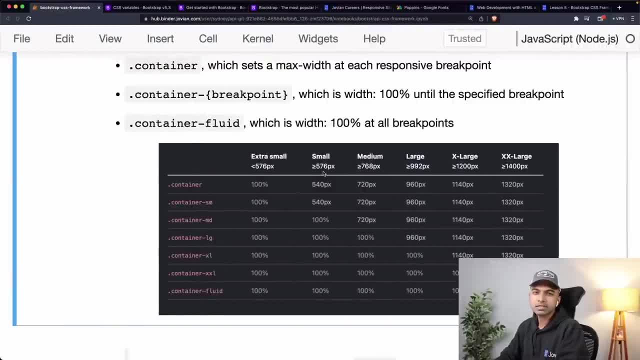 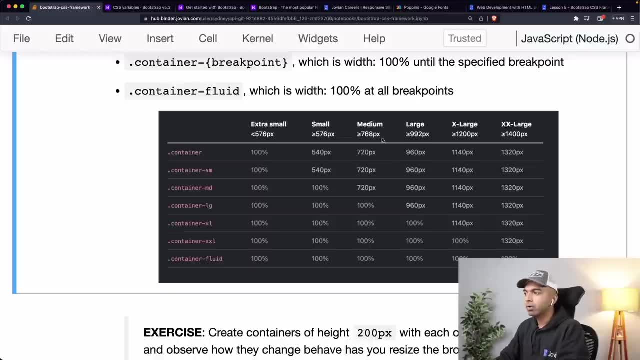 width. No till about 576 pixels. it's going to occupy the full width. Now, at more than 576 pixels, it's going to be 540 pixels. At more than 768 pixels, it's going to occupy the full width. 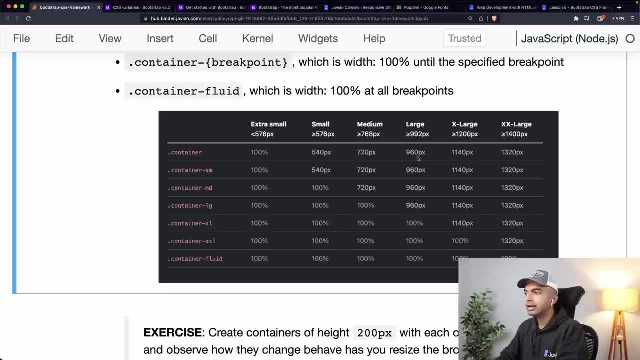 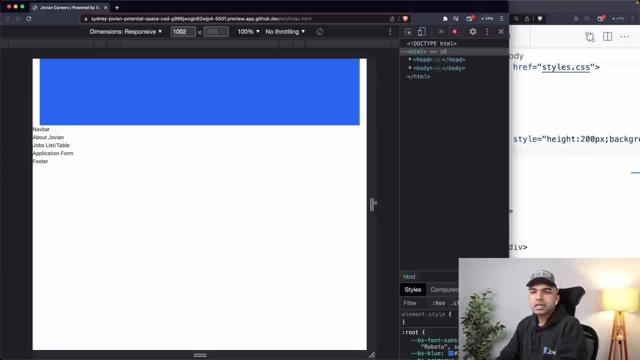 At more than 668 pixels, it's going to be 720 pixels wide. at more than 960 pixels, it's going to be 960 pixels wide, and so on. Okay, so it just gives you a nice centered div, or horizontally centered div on the page. 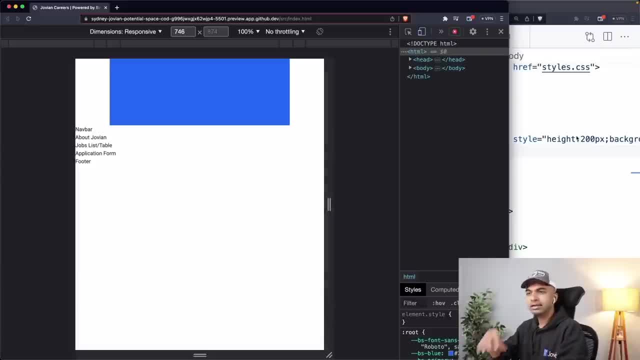 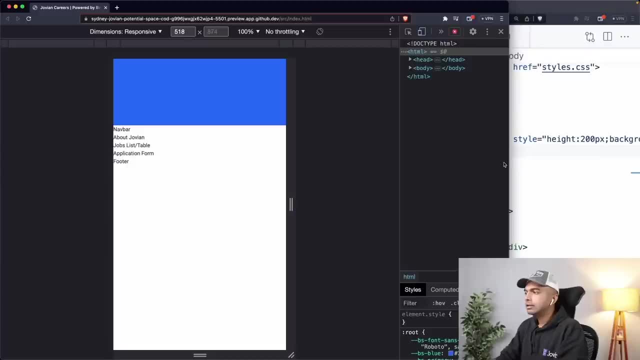 and you can put all your content inside this div. Okay, so the container is going to contain all of the rest of your page content. Now, of course, you may not always want this. what you may want is: maybe you may want it. 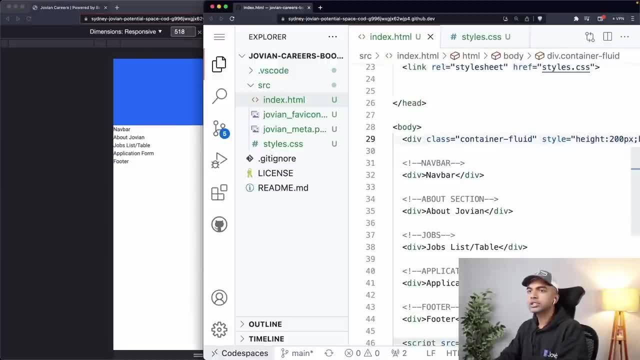 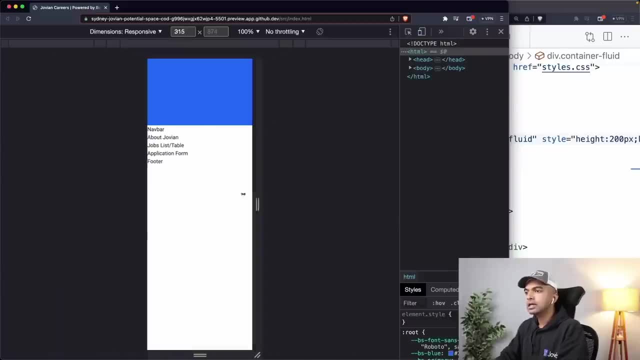 to always occupy the full width. if you want it to occupy the full width, just use the class container fluid. If you use a class container fluid- and let me reload that page- If you use a class container fluid, then it's going to always occupied the full width of. 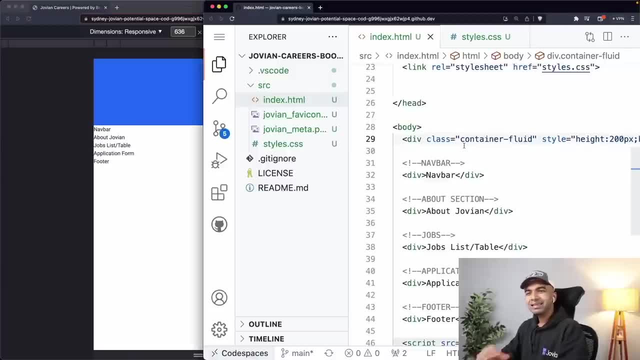 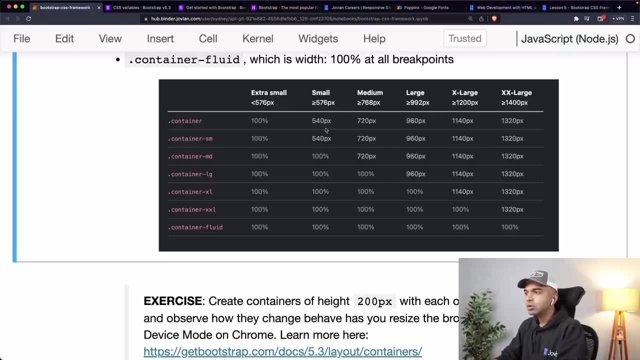 the page. All right, that's container fluid, And then there are various steps in between. you could do something like this: you could say container SM, And if you say container SM, so up to the highest point of SM, which is just before. 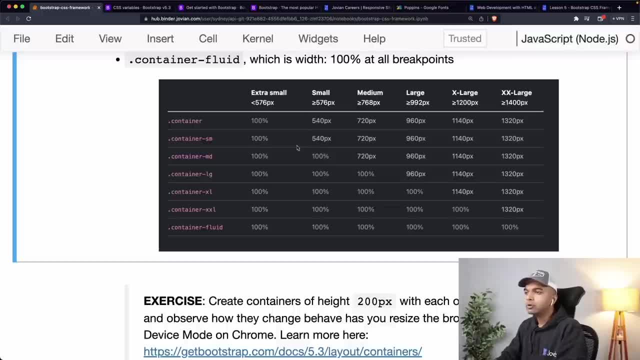 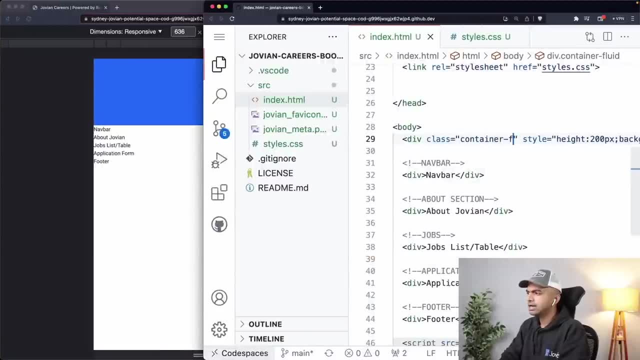 MD. it's going to probably still use up okay, or up to the size SM. it's going to use up the full width, So from the size SM it's going to become centered okay. So container SM- I think it's going to do the same thing as container for us up to 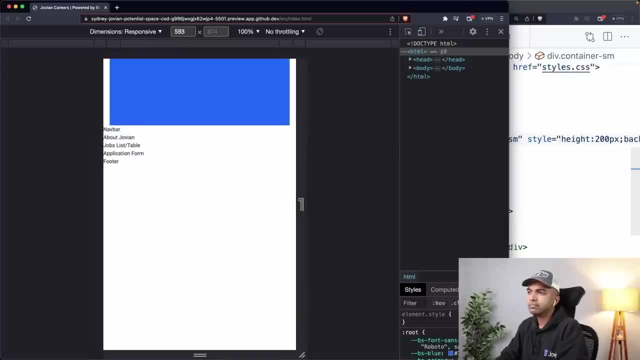 540 pixels. it's going to take up the full width at 560, or 576 pixels. it's going to become centered. you can also use container MD Now. container MD is going to take up the full width till 768 pixels, and it's 768 pixels. 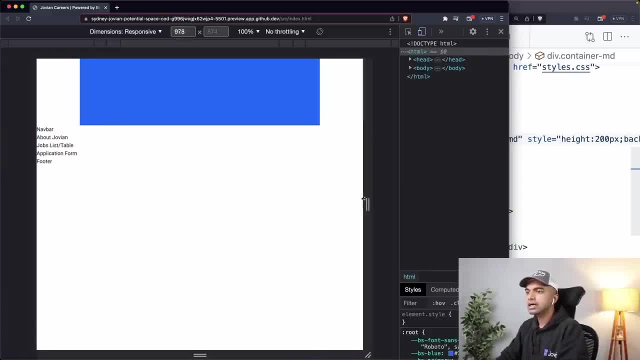 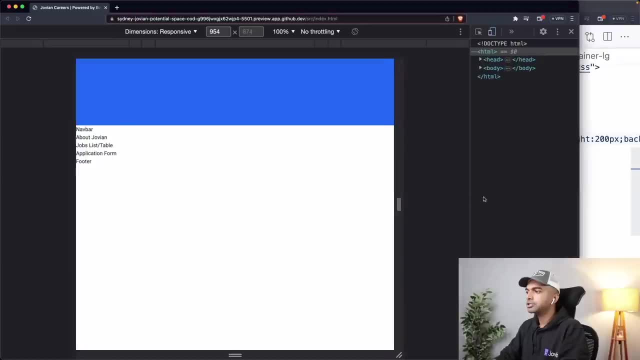 it's going to start restricting its width and progressively increase size with breakpoints. Similarly, you can do container LG, Which is going to use up the full width up to a certain large size and then, after a certain point, is going to use the center. okay. 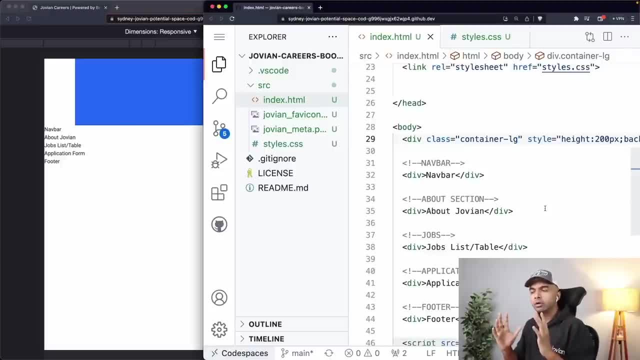 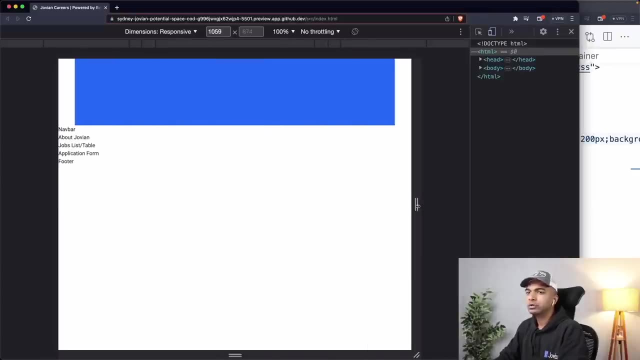 So, depending on when you want to constrain the content of your page, you can decide which container you want to use, And for now I'm just going to use set it back to div container, And what that is going to do is, given no matter what width I'm at, is going to just center. 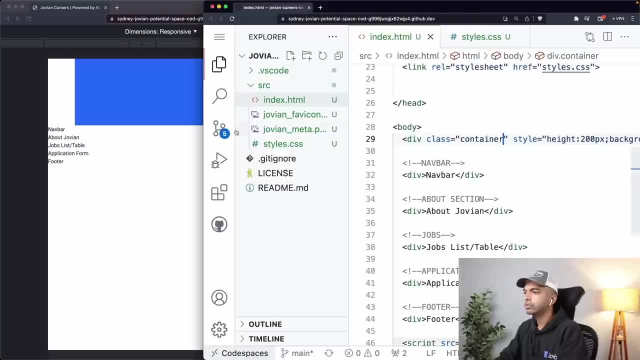 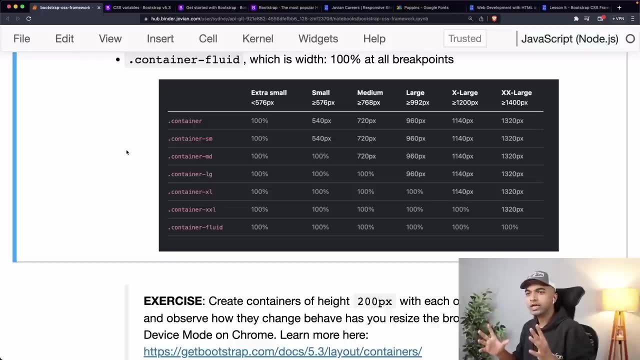 the content a little bit on the page, have some padding left and right. Okay, so that is the container. that is the first basic thing. no matter what you're doing in bootstrap, what, whatever page you're building, the first thing you'll probably do is just: 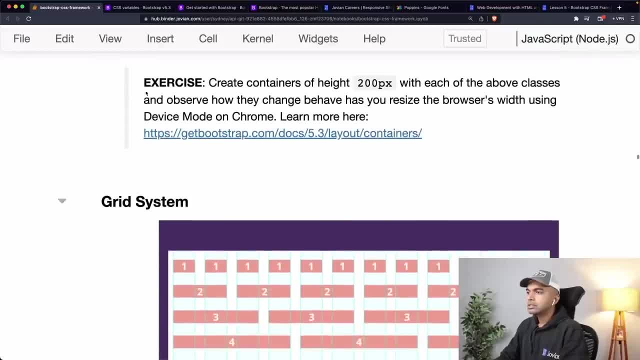 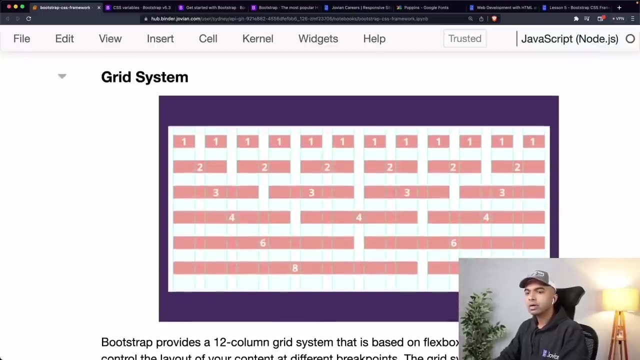 create a container. Okay, so one thing you can do as an exercise is maybe create a bunch of containers one below the other and give them all different container classes and see what happens to each of them as you resize the page. Now, the next thing that we need to understand, once we've talked about containers, is the 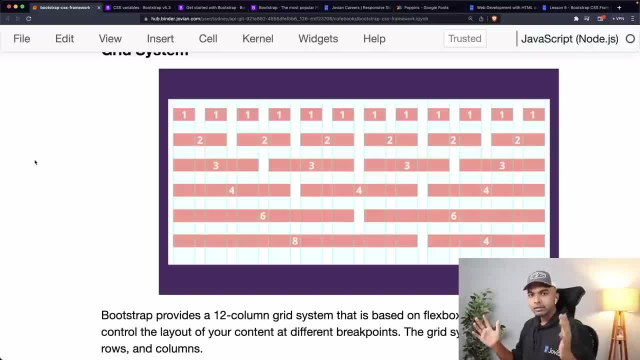 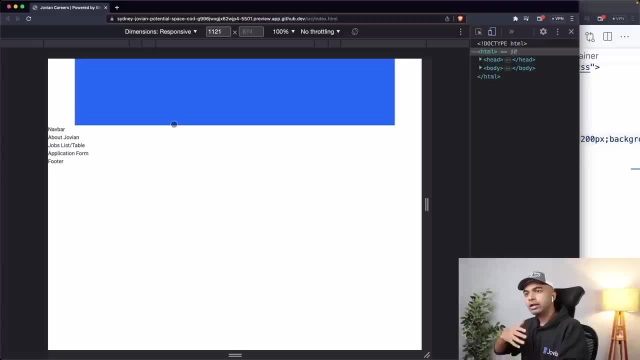 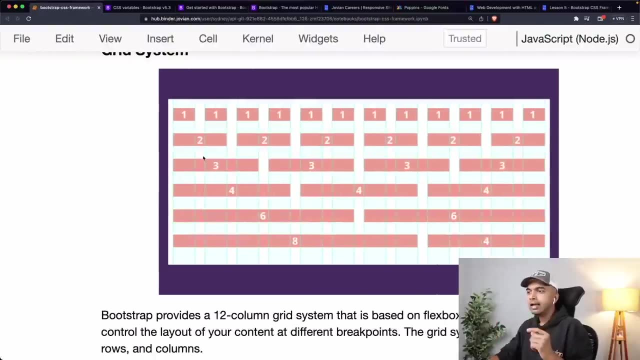 grid system, So every container contains 12 columns. you cannot actually see these columns right now, But every container is inherently or internally divided into 12 columns, And then what you can do is you can decide to put content and you can decide how many. 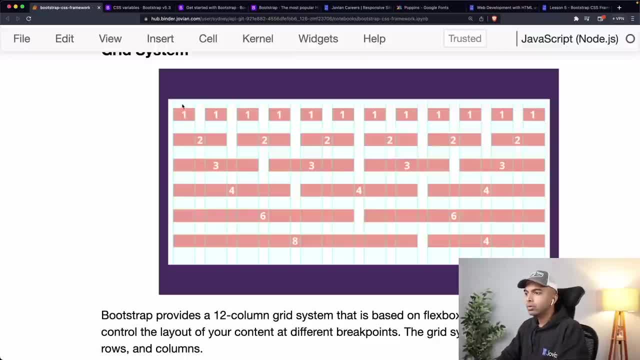 columns that content can take up. Okay. So here is an example. you can. you can just maybe have a bunch of dips. you can have maybe 12 dips. each of them takes up one column and there is also some space between the columns. 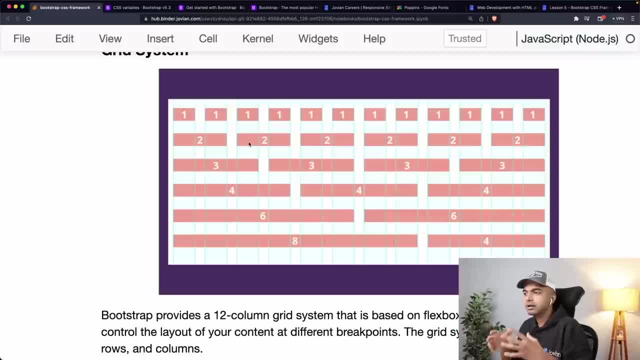 or you can have something like two dips and you can have six of those dips taking up six columns, Or you can even combine things. you can maybe have a div that takes one column. you have a div that takes two column next to it, a div that takes some more columns next to it. 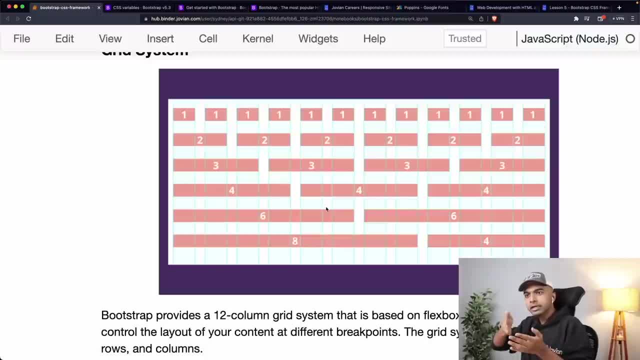 and so on. Okay, so, whenever you need to horizontally arrange columns in a row, or so, whenever you want to arrange divs in a row and you want to control their relative width, that is when you use this grid system. And the grid system is invoked using two cleats. 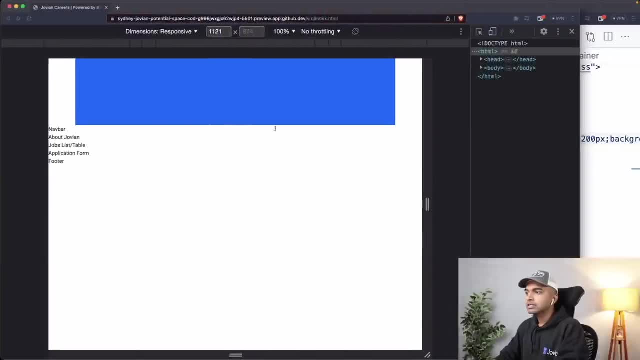 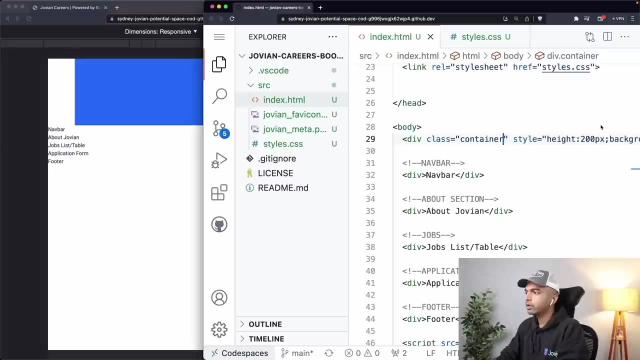 Okay, There are two classes, So the first class is the row. So let's say you want to create three divs here. you want to create three divs and each of those divs should have an equal width. So here's what you can do within your container. 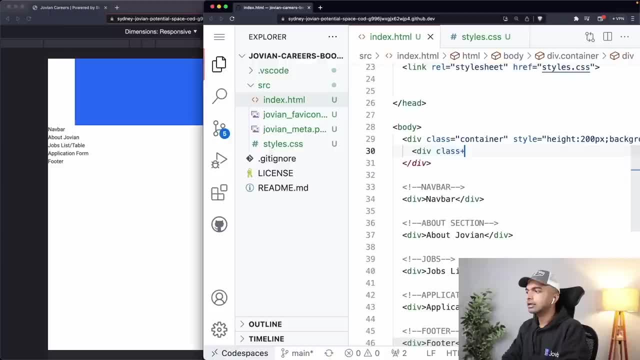 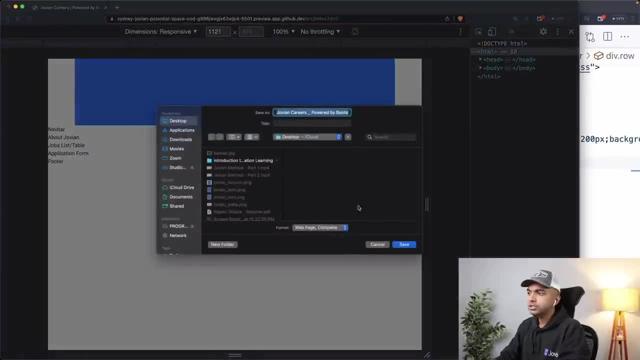 Remember, all of this always happens within a container. create a div with the class row. Okay, Now we've created a div with the class row. nothing has changed here. Yeah, nothing has changed here. Now I can create a div with the class. 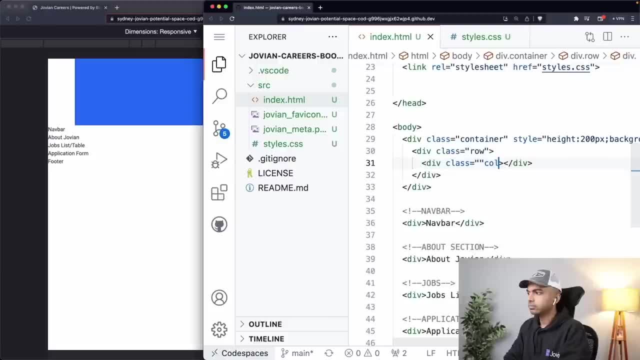 Column. Okay, and let me just call this box one, And let me also maybe give it a border. Let's get a nice solid black border And let's create a couple more divs like this. Okay, so I'm simply creating a few. 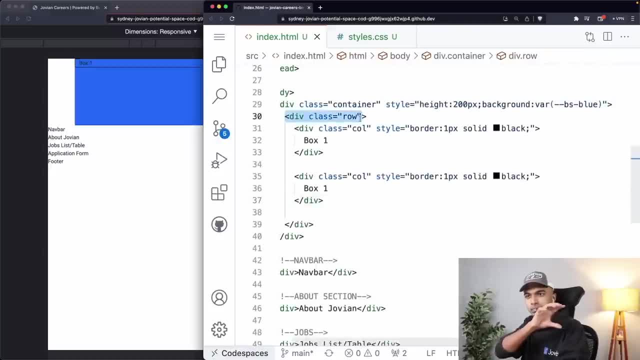 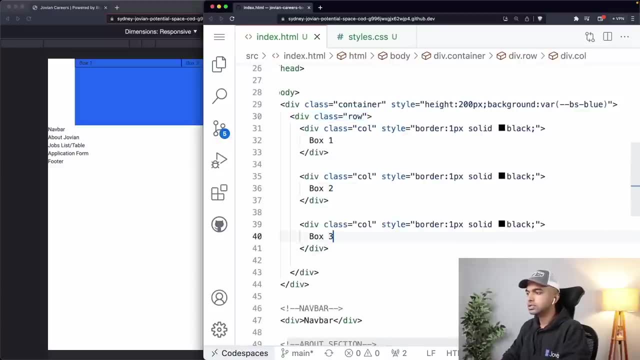 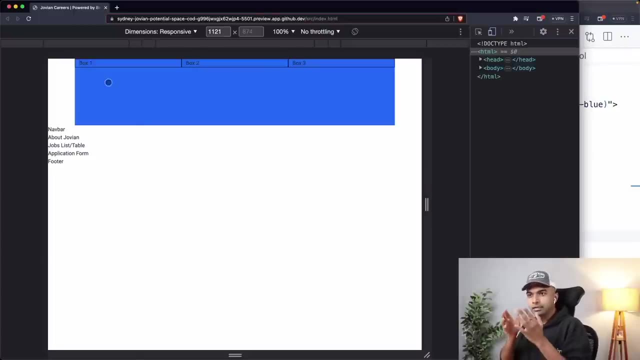 I've created a row And that is going to simply put things in a vertical order. Then I'm going to create a bunch of boxes here, box two and box three, Okay, And let's see what happens. So you can see now that we have taken the container. 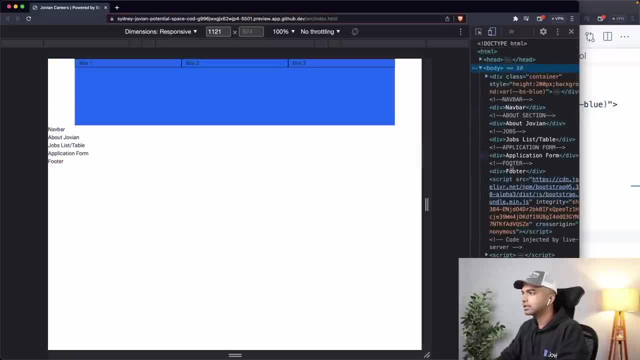 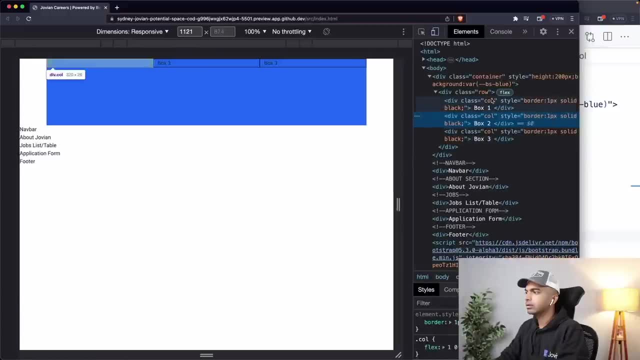 And then there is this row div that has been created And I can just go in and actually get to that row div here as well just by selecting inspect element. Yeah, so there is this row that has been created And then within that row we have these three columns: 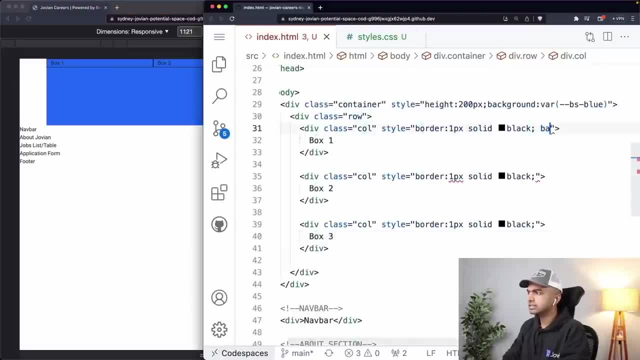 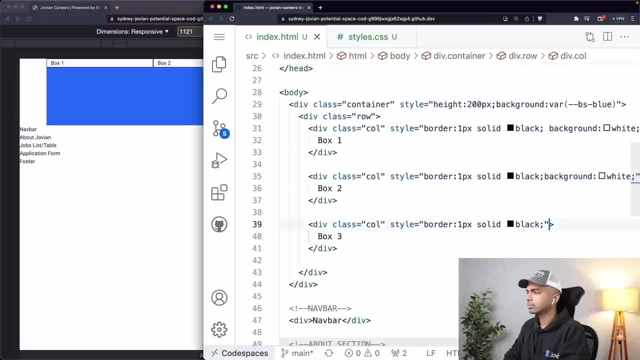 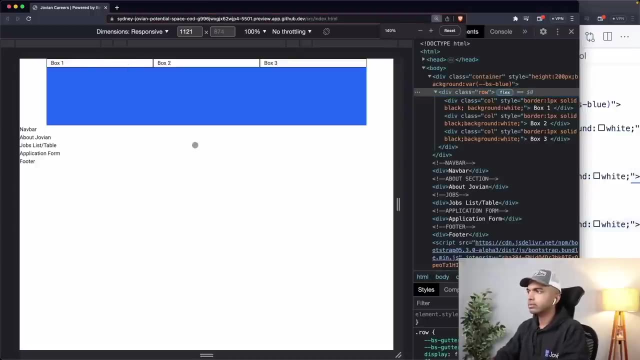 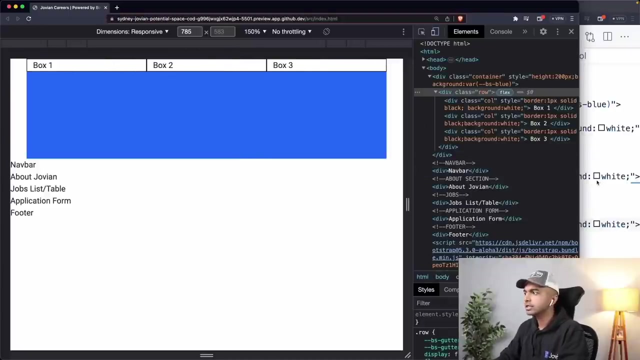 Let me just make the background white for these, just so that you can actually see these clearly. Yeah, so within the rows, we have these. within the rows, we have these three columns. okay, box one, box two and box three. 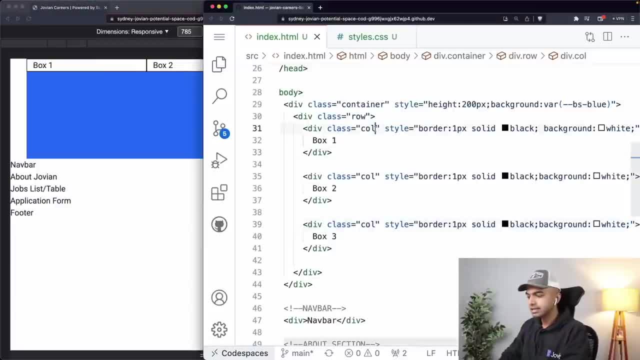 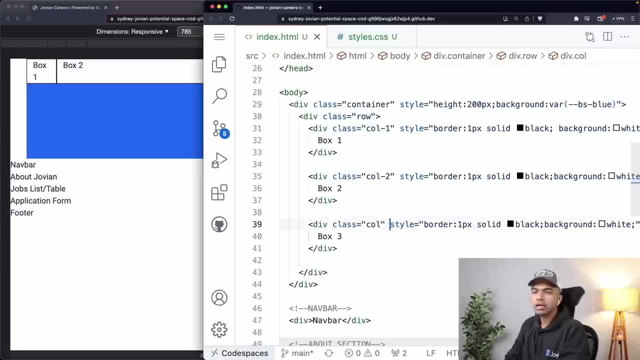 Now something I can do is I can actually specify ratios for these. I can say call one, which means I'm wanting to take up one out of 12 columns, And I can say call two, I want this to take up two out of 12 columns, and I can say: maybe. 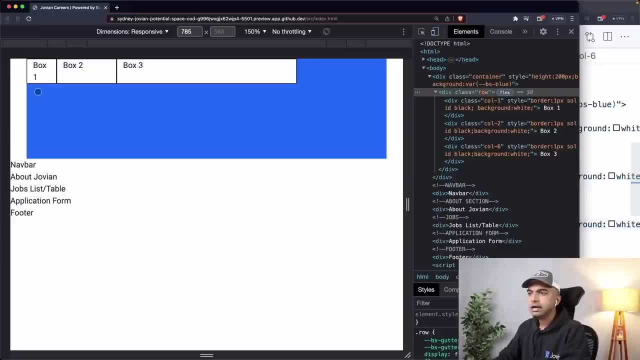 call six. So now you can see that I have this box one which takes roughly 1, 12th of the space available in that row. Okay, this is the entire row and it takes up 1, 12th of the space. 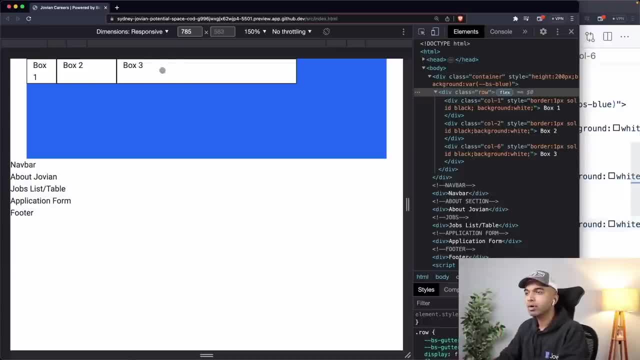 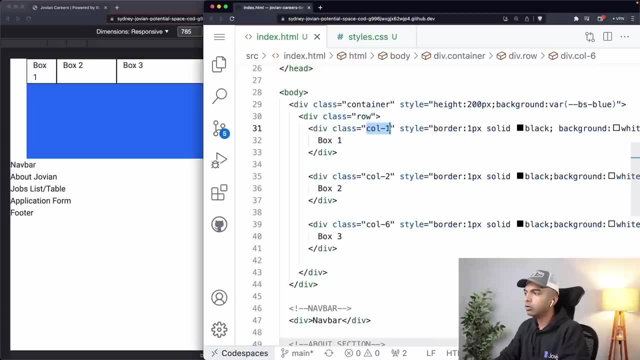 Box two, on the other hand, takes up to 12th or one sixth of the space, and box three takes up six columns, right? So imagine there are 12 columns here And what we've specified here is call one or two and call six are the relative column. 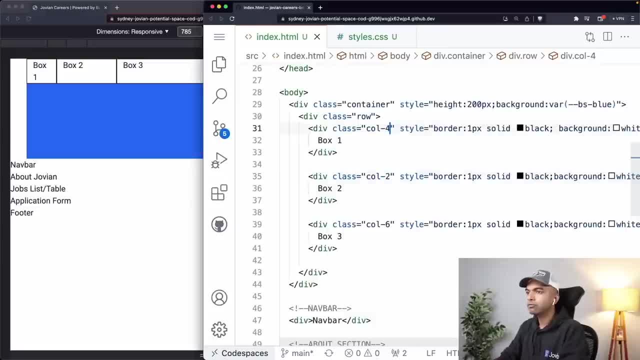 widths. that should be taken up. Now, of course, I can play around with this. let's say I want four columns for row one, And then I want two columns for this, So four plus two, six, and then the remaining half goes here. 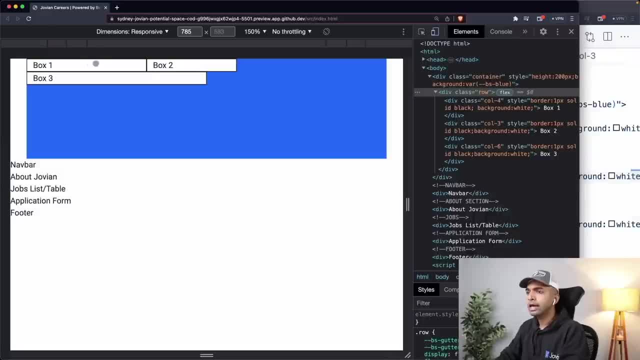 And let's say maybe, what if I had three columns? What would that do? So now you see what happens when I have four columns here plus three columns here, So that becomes seven, seven plus six becomes 13. And then the next column automatically drops onto the next line. 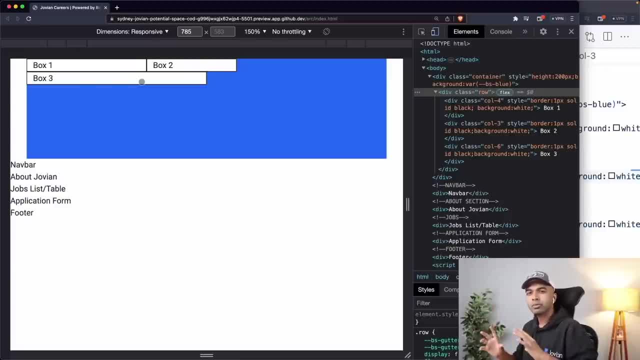 Okay, so it's using flexbox internally, but you don't have to worry about flex basis, flex grow, etc. You just tell it how many columns, how many columns should be taken up by a particular box, and it's going to automatically arrange the widths and if the number of columns in 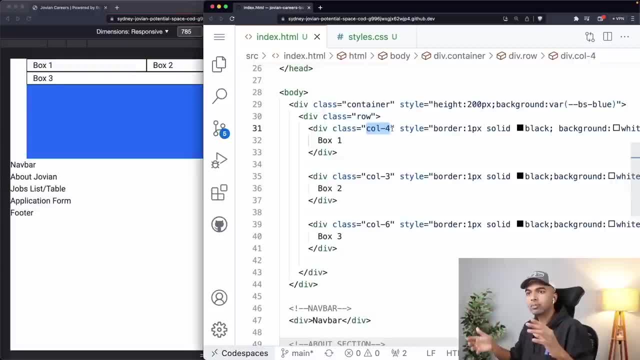 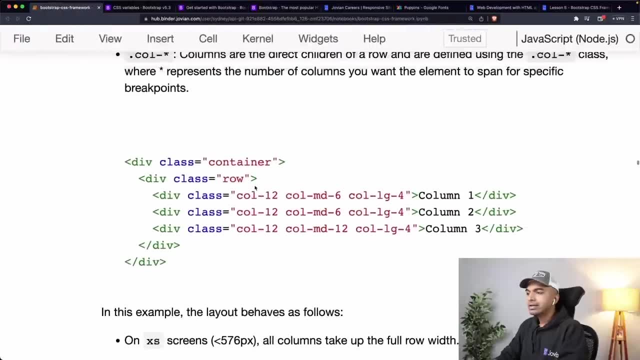 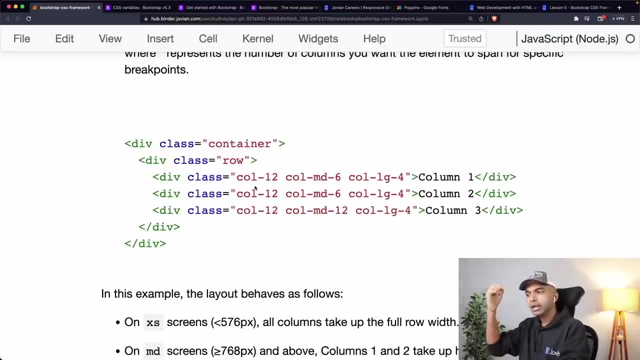 a particular row goes higher than 12,, then it's going to drop down into the next next line automatically. Okay, Now where this gets a little more interesting is that you can actually modify the widths of each of these boxes based on the breakpoints. 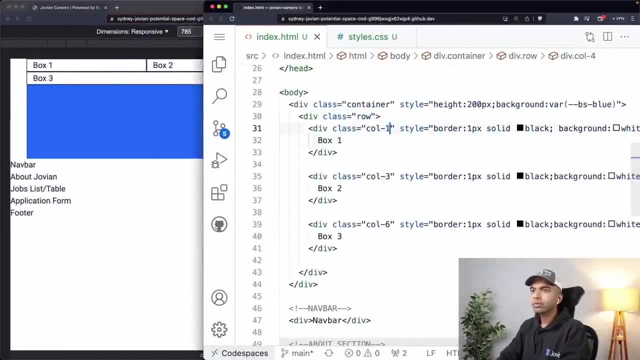 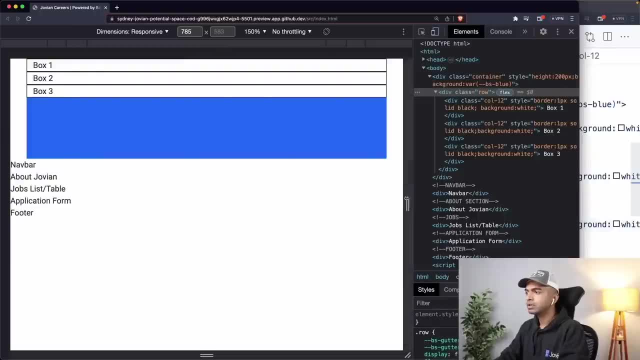 Okay, so we can start out like this. we can just say: call 12,, which means we want box one, box two, box three, all of them to take up all 12 columns. okay, So no matter what width I'm at, it is going to take up the entire width of the row. 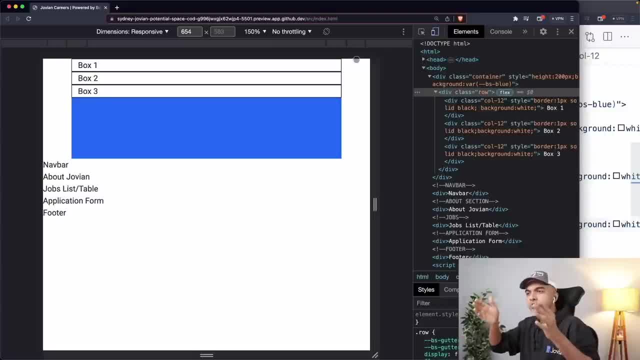 And that is why So it's, it's supposed to be a row, or because box one takes up all 12 column, box two drops onto the next line, box three drops onto the next line, and so on. right, So this is fine. 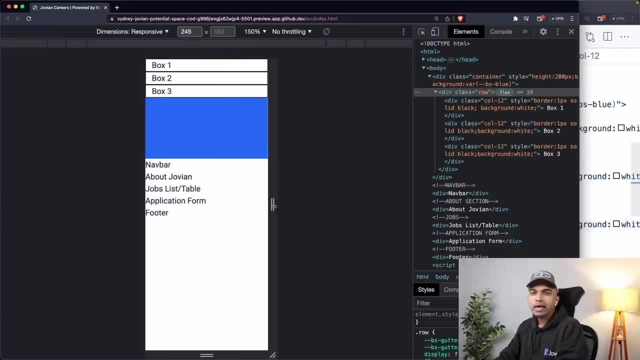 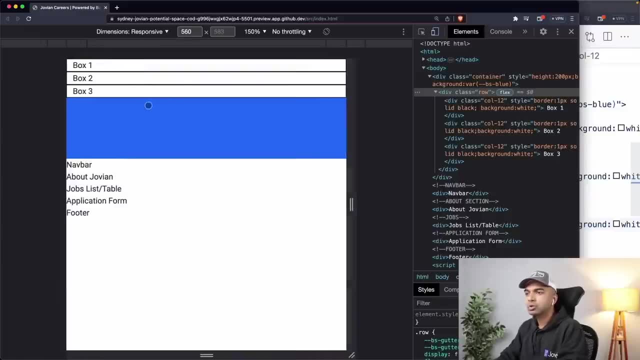 But maybe when I get to- and this is maybe nice for a mobile layout- I want to show three things one below the other, But maybe when I get to a tablet or MD layout, I want to show maybe box two and box three together or some other layout. 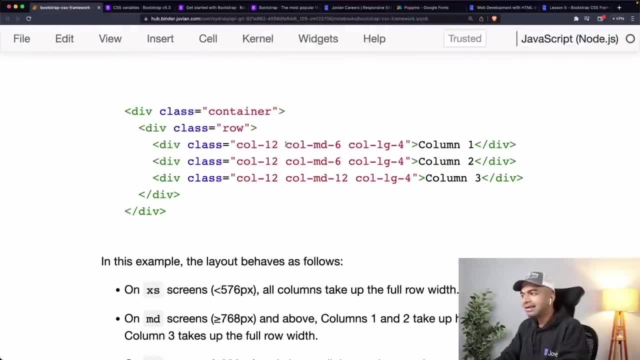 So then you could do something like this. you could say that okay at MD. so you can say: call hyphen MD. So what you're saying is, when we hit the MD breakpoint of 768 pixels, I want box one to take up only six columns. 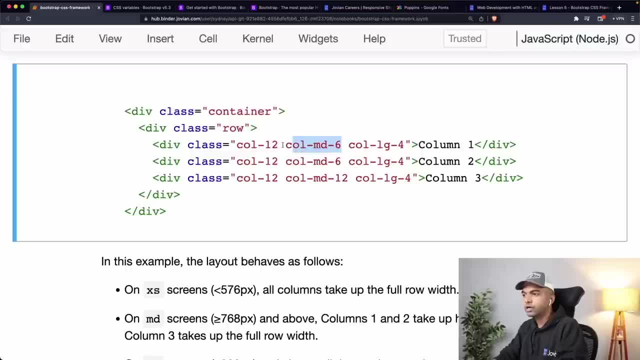 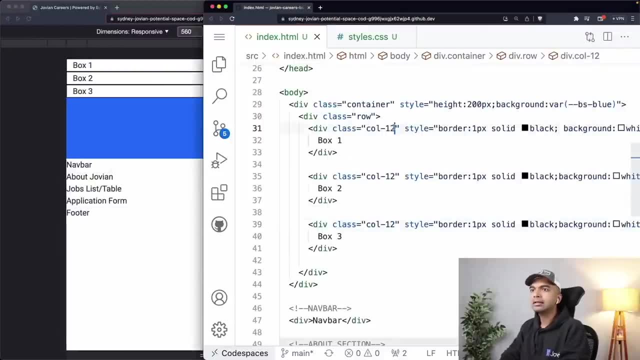 Okay. so remember, we are going mobile first. So first everything takes up 12 columns. But now I want box one to take up six columns. So I'm going to come back in here and I'm going to add the class call MD six. 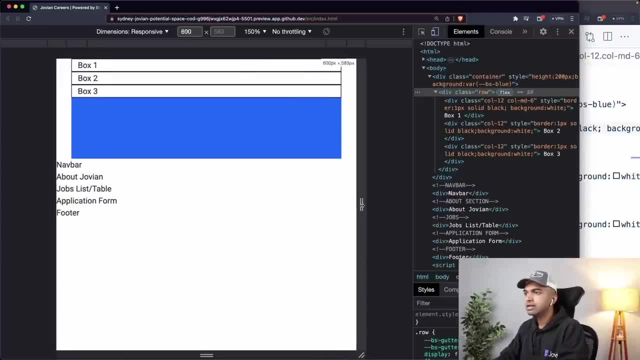 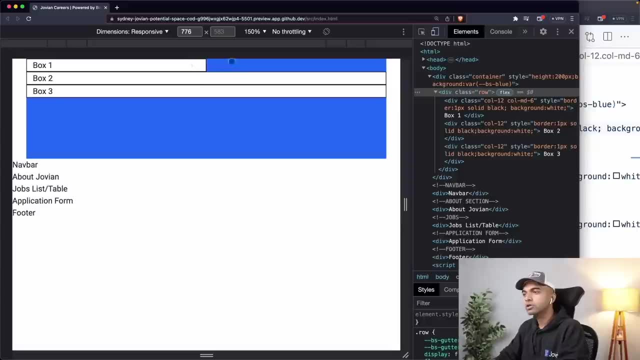 And with that you will see that as soon as I cross 768 pixels box one, It starts taking up only six columns and not 12 columns. Now, of course, box two is still falling onto the next line because there are not enough. 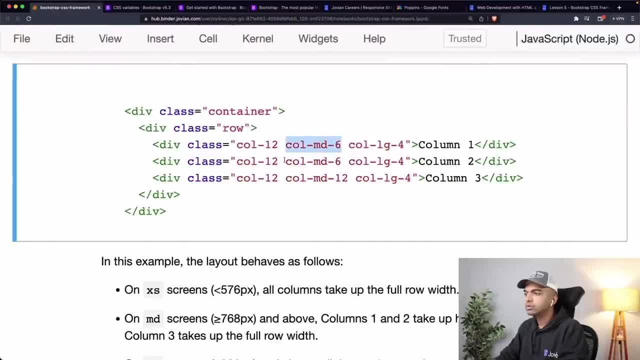 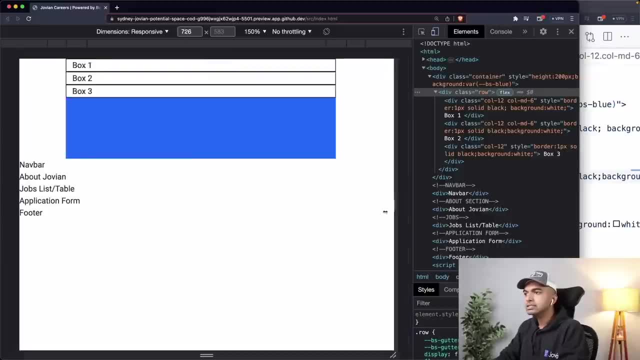 columns to fill its 12.. And maybe then, once again, we want to use six columns for box two as well. Right, And now you see what happened: that up to 768 pixels, all of them show up one below the other, But as soon as we go into 767 or 769 pixels, box one and box two come up side by side. 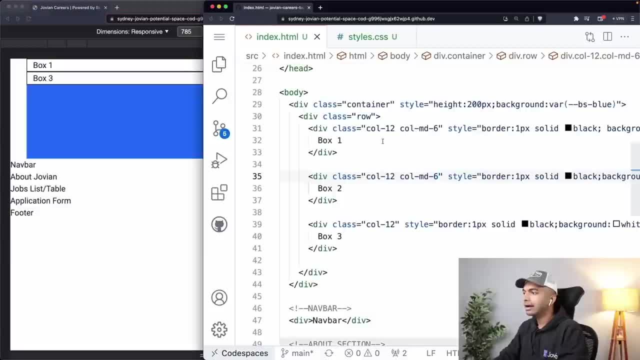 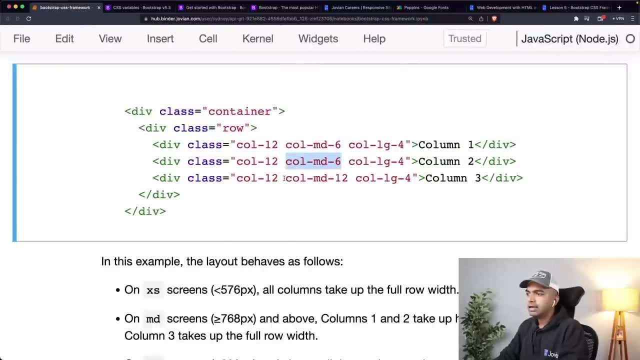 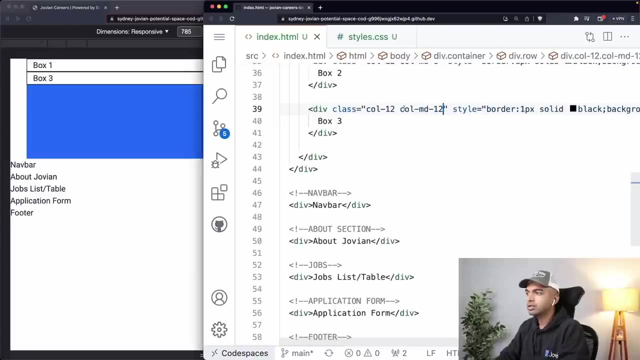 The reason they're coming up side by side is because we have overridden the property at this breakpoint, using call MD six and column D six And at maybe at MD we still want to retain 12 for the third column. So we don't, technically we don't need this property because it's simply going to carry. 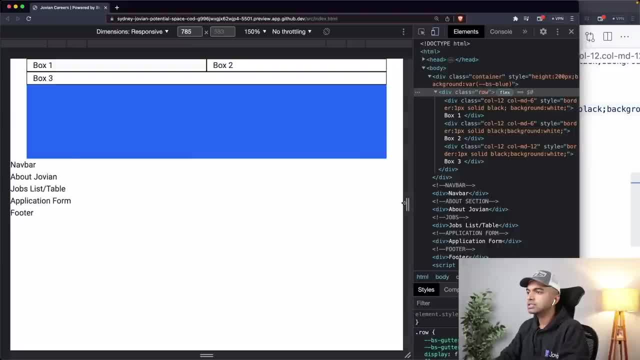 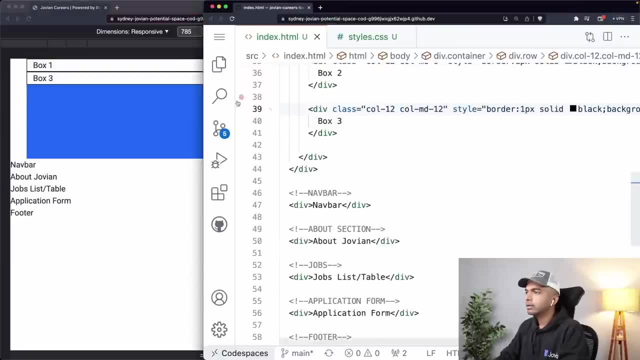 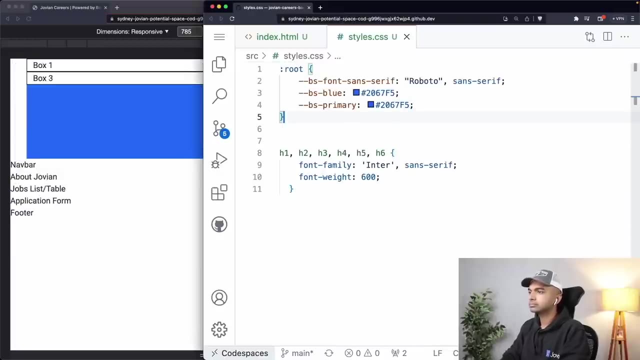 over from whatever is there here. So whether I keep this or I don't keep this, it's not going to make a difference. It's box three is always going to take up the full width. Now Let me also increase the body font size a bit. 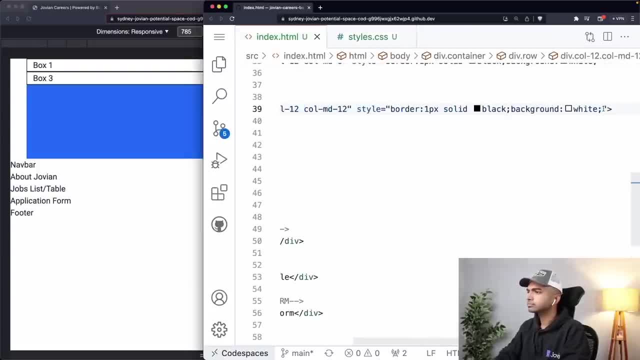 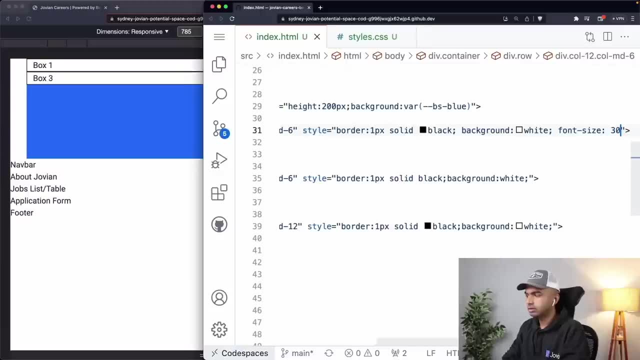 Let me just increase the font sizes of the columns. Yeah, So that our columns are a little bigger. I'm just using font sizes of 30.. Okay, Perfect. So now I have box one, box two and box three, And this is on MD. 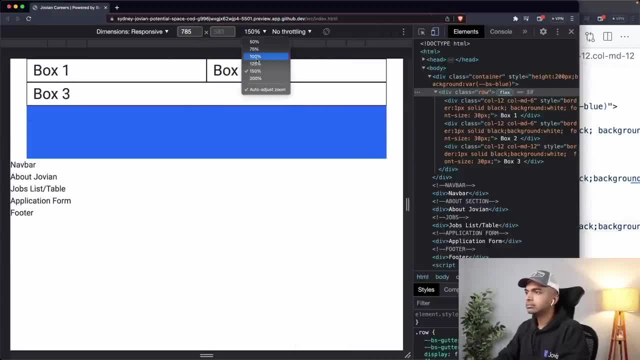 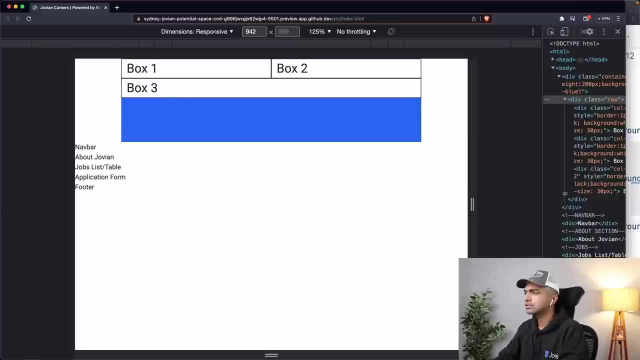 And now, at some point we are going to now hit maybe the next layout, which is going to be LG, right? So LG is going to be about 968 pixels and 992 pixels or so. So there's no change yet, but maybe on a very large screen I want to show all three columns. 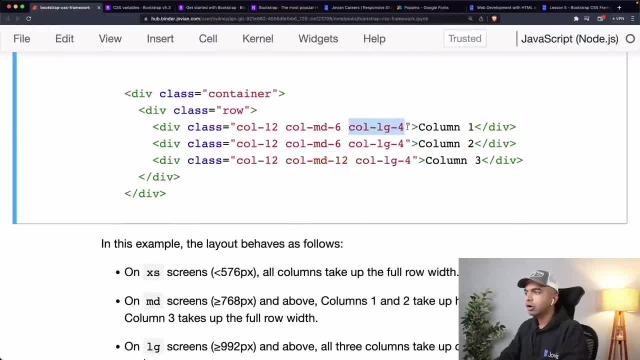 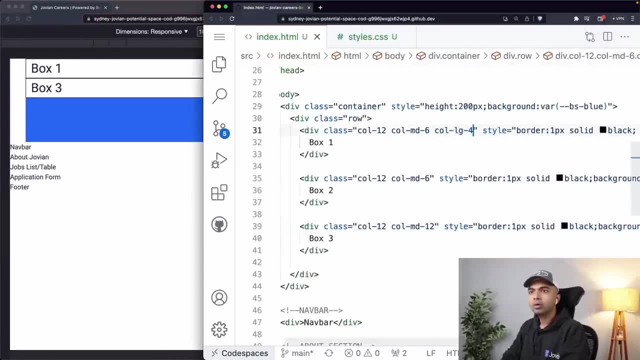 side by side. So in that case I can do something like this. I can say: call LG four, and I can apply that style to all of them. So let me go into The first box, First box and use: call LG four. 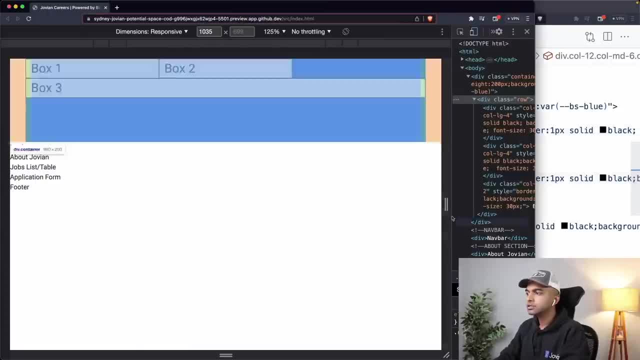 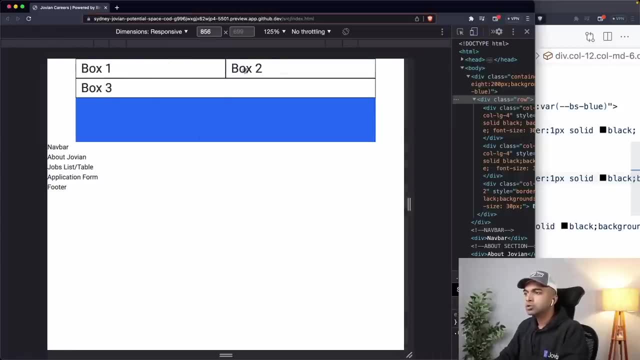 Let me go into the second box and use call LG four. You can see now that as soon as we crossed about 906, 996 pixels or so, Now box one and box two are no longer taking up half of the row, They're only taking up one third of the row, which is four out of 12 columns. 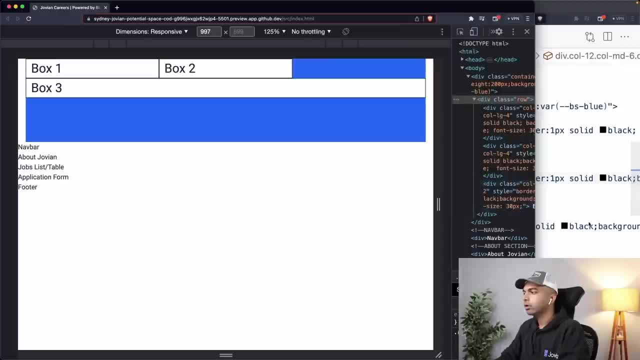 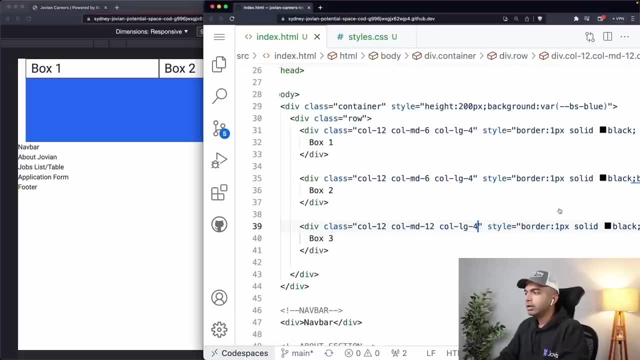 And now we can maybe take box three and put this here on the corner. So let me also apply all LG four, and now box three shows up here as well. Okay, So to do this in a slightly different way as well, we can maybe use call LG three for 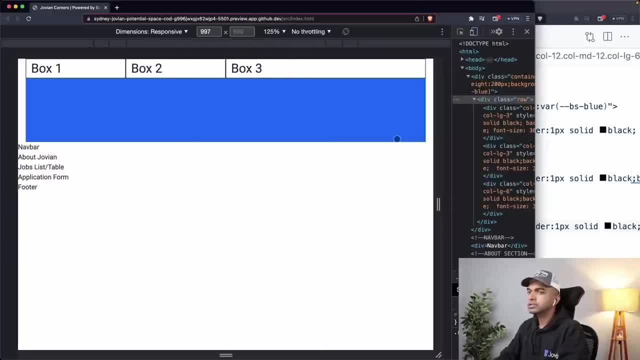 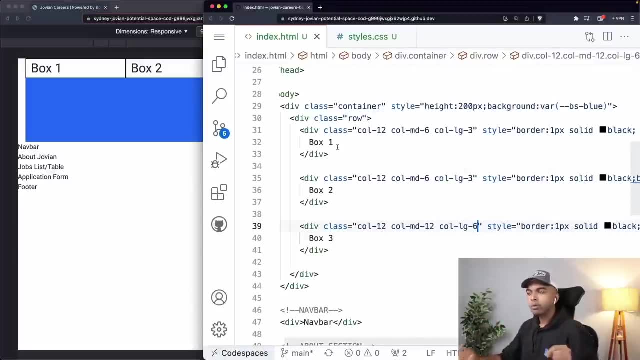 the first two boxes and maybe six for the third box, because the third box may have more content. So now you see what we've achieved. We have not written a single line of CSS, but we've achieved this very interesting layout where first we have box one, box two, box three, all three of these, and you can put 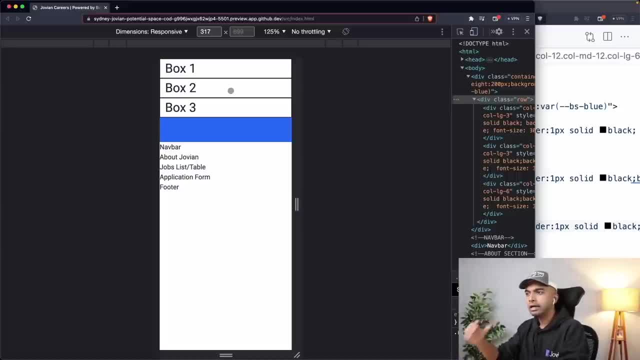 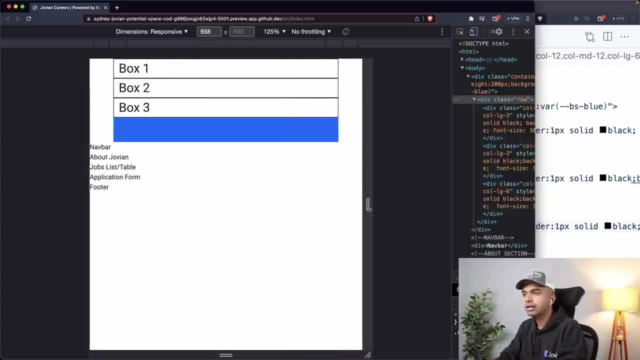 any content inside this, maybe an image, a heading and then and then some text, And then, as soon as we- or maybe a heading text and then some content, as soon as we go into the tablet layout, which is about this much, then box one and box two come. 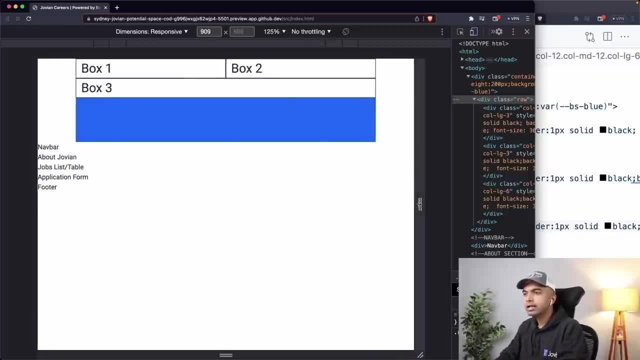 up side by side because we have more space now, So we can do that. And as soon as we go into LG, then box one, box two, box three all show up side by side and they have the proportions that we need. 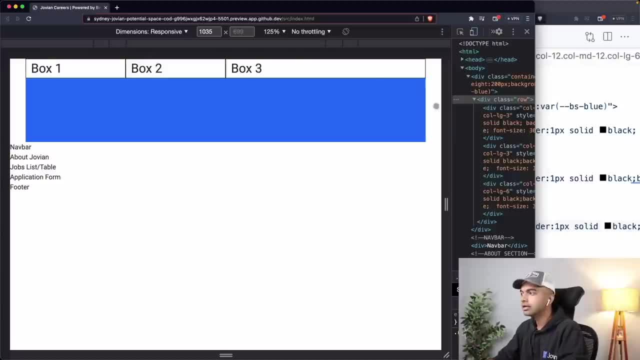 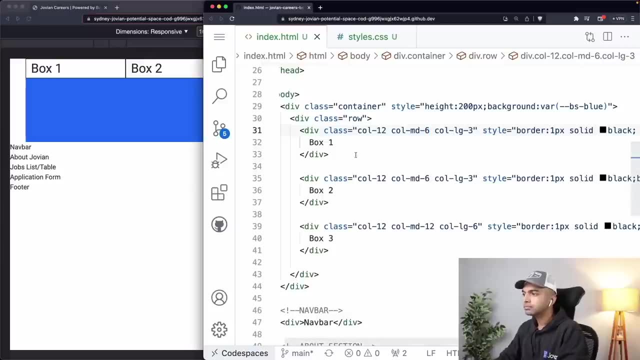 This is very, very powerful, And if you can master using bootstraps grid and if you can know what are the right properties to use here, then things are going to become really, really easy for you. Okay, So that is the bootstrap grid system. 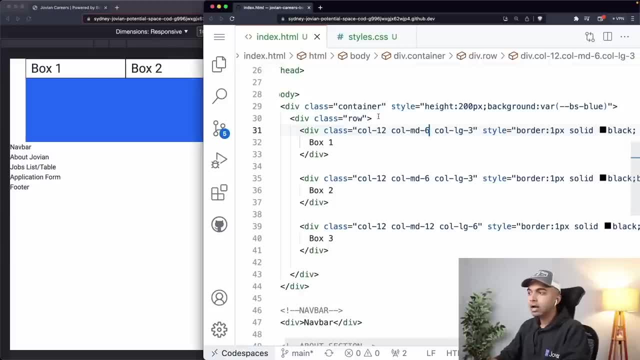 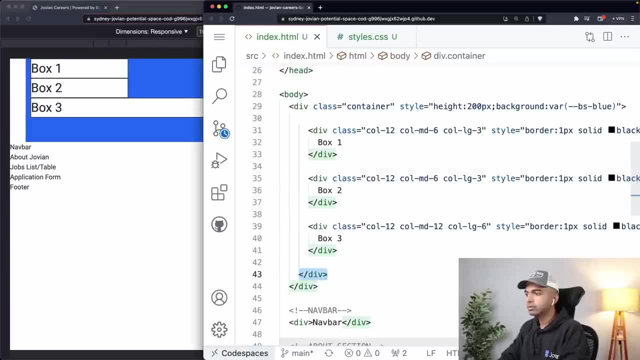 Using rows and columns. Now, one thing I want to mention here: that you have to have this row If you want to put things into a column. okay, If I don't have this row class here, then every all the devs inside the container are. 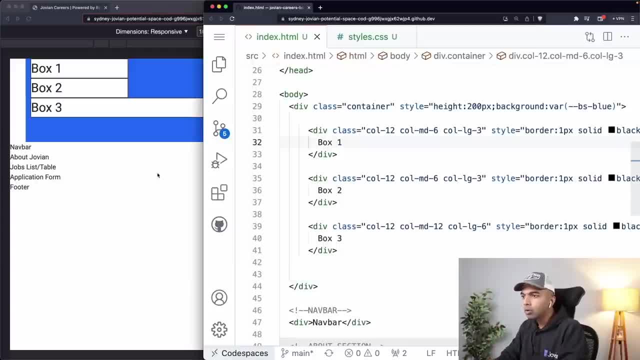 going to be one below the other. You cannot avoid that, Although the column, the number of columns that pick, is still going to get picked. So box one is picking three columns, Box two is picking three columns as well, And box Three is picking six columns. right, 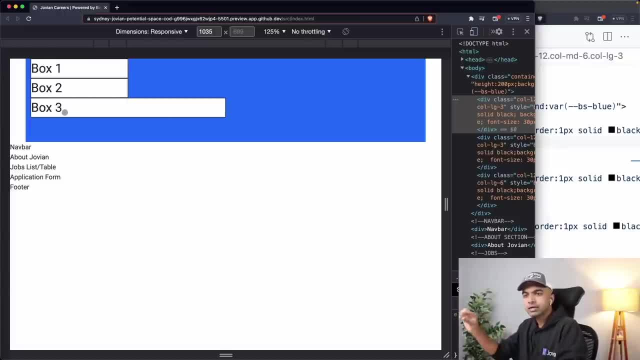 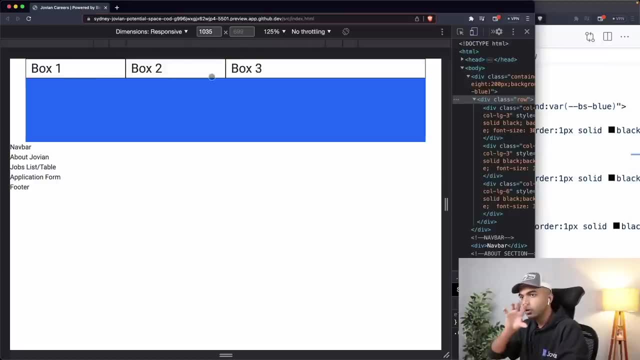 So that's, they're picking up the right weights, but they're not showing up in a single row, because to make them show up in a single row you have to drop them or you have to wrap them in a particular row. dev, Okay. 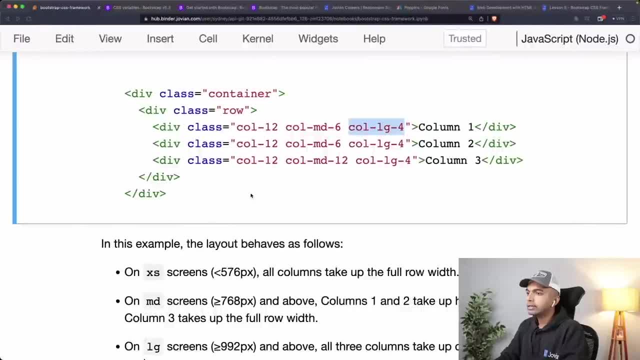 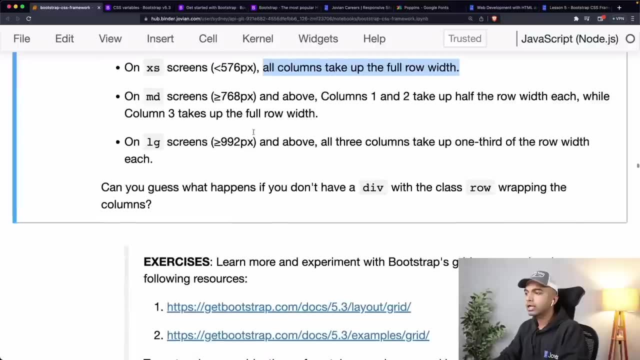 So keep that in mind, All right, So that is the. that is how this behaves on excess screens. All columns take up the full row width and show one below the other. on MD screen seven, 68 and above, column one and two take up half the row width, while column three takes up. 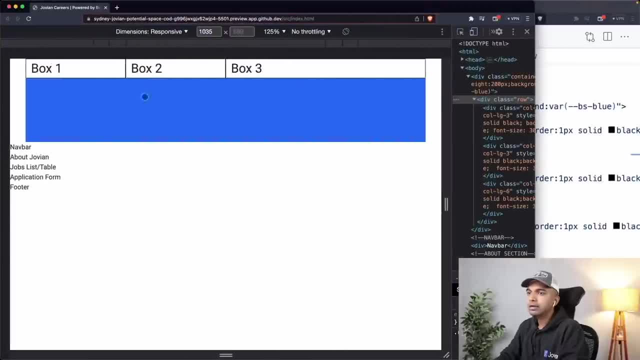 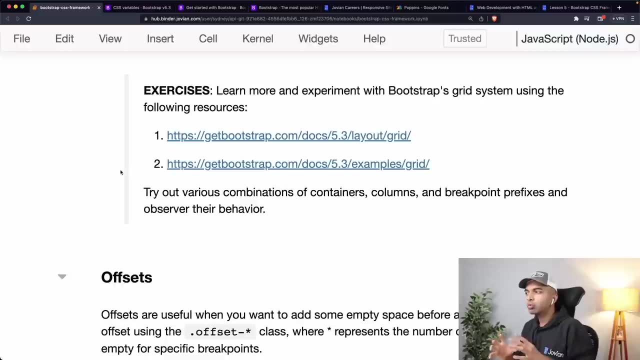 the full row width and on LG screens, all three columns are on the same row and we can decide what are their relative proportions. Now I would encourage you to experiment with bootstraps grid system. So there are a couple of resources you can check out. 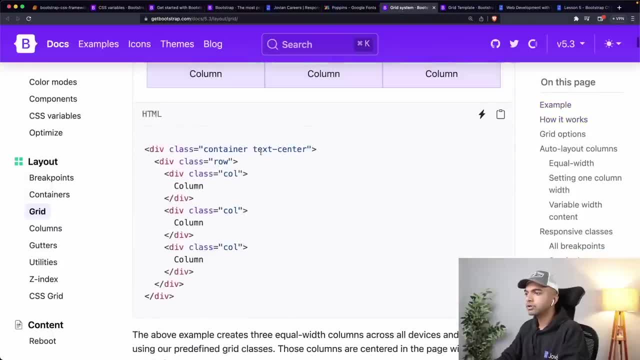 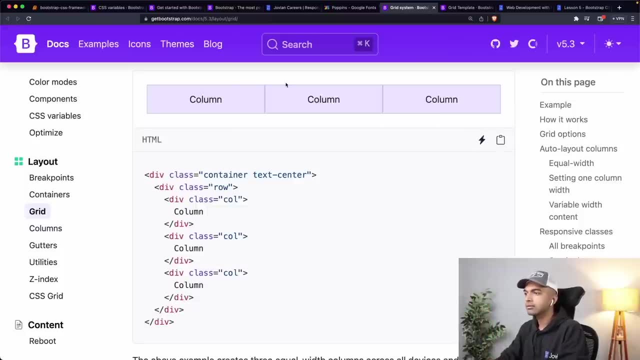 One is the documentation itself, and it has a bunch of different examples and you can just click this button and live edit these examples. So it's going to open up a cloud editor for you and you can start editing. This is, of course, the equal layout, but you can also have these unequal layouts like this: 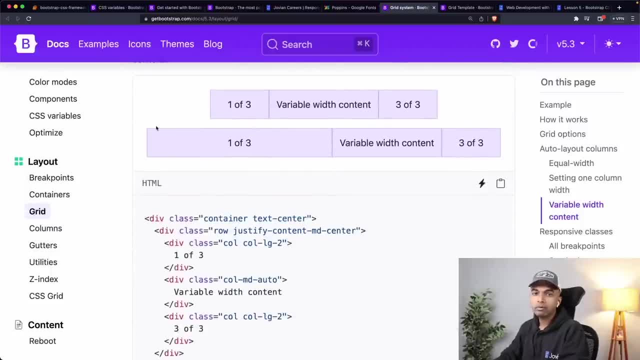 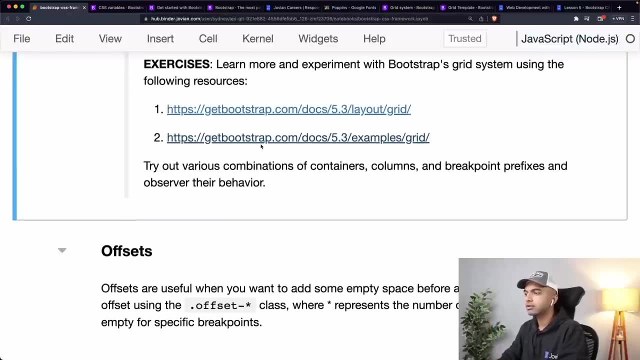 And you can do a whole bunch of things, So I would encourage you to experiment with this. There are also a bunch of examples that are given along with the documentation, So you can check these out as well. Okay, Make sure you get a strong, a clear understanding of how the grid system works. 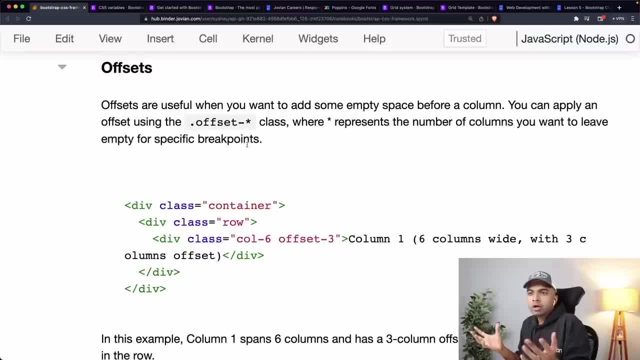 Now, apart from this, you can also- sometimes you may not need a column on the left and a column on the right, You may just want to maybe just shift a particular column a little bit. So then you can also use something called an offset. 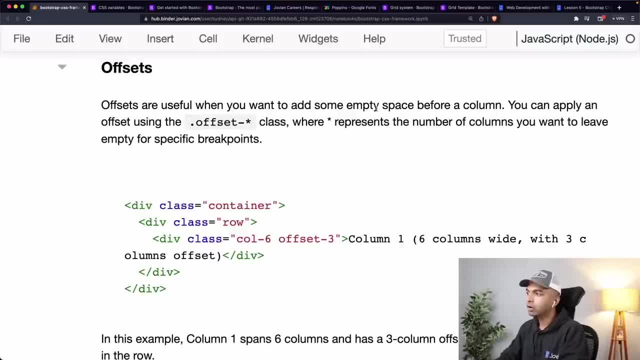 So an offset is useful. Okay, You can add some empty space before a column and you can apply an offset using the dot or using the offset star class, where offsets represents the number of columns that you want to leave empty for a specific breakpoint. 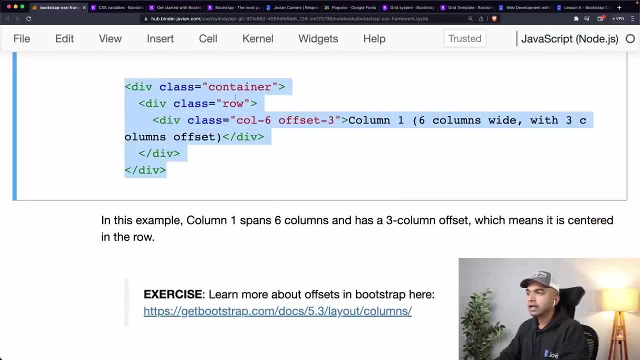 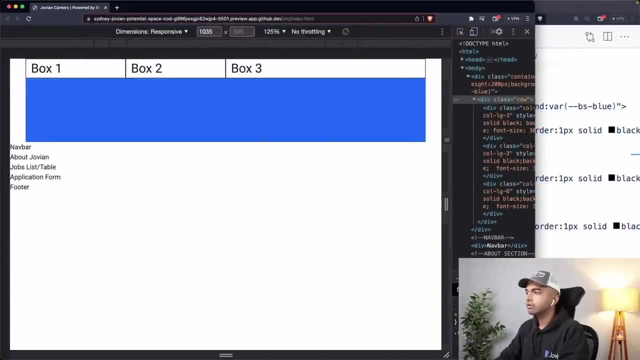 For example, we could have something like this: We have a div and we have a container inside it. We have a row and inside it we have just a single div. Okay, Now we don't have multiple divs, We have just a single div, and I'm actually just going to copy this class from here: 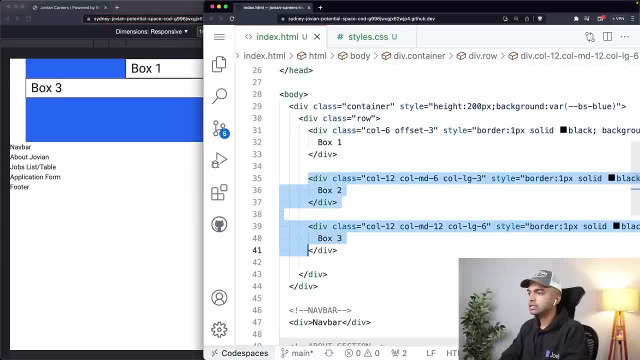 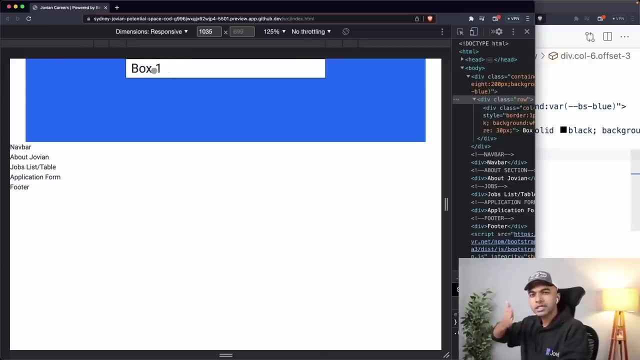 And I'm going to get rid of all of these. So now I have a row, but what I want is I want this box to only take up six of the columns and I want it to leave three columns on the left, And that is what the offset does. 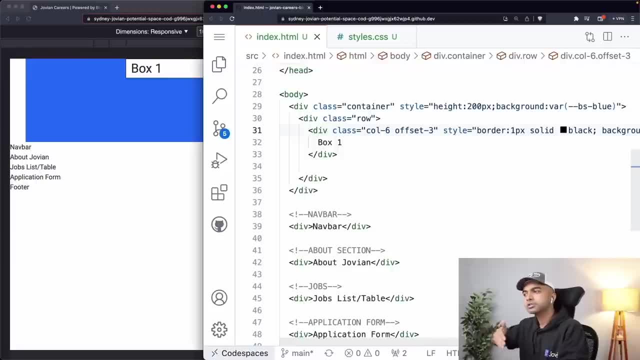 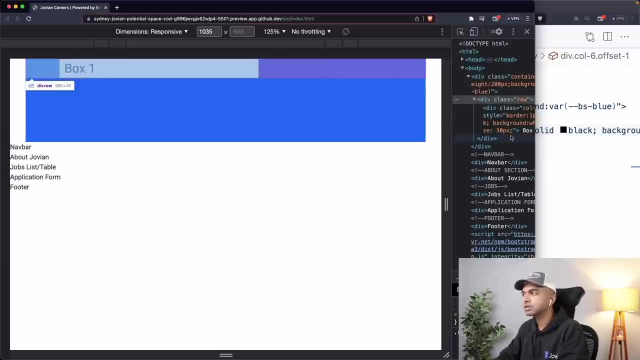 So when I say offset three, it's going to leave out three columns on the left and it's going to start from the fourth column. If I said that to offset one, you can see that it leaves one column here empty and it then span six columns. 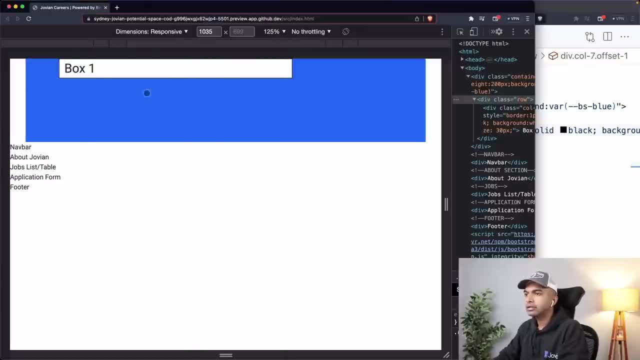 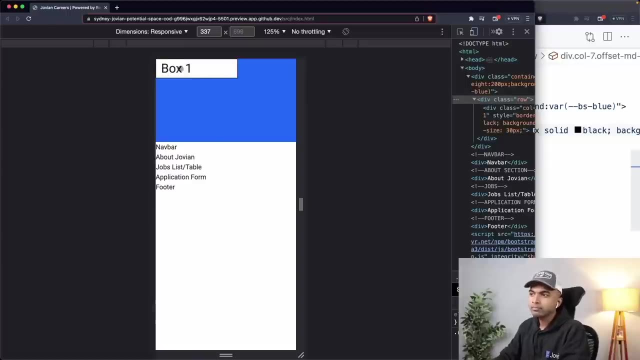 I can of course then maybe set it to call seven And you can see that it actually does that, And I can also then play around with breakpoints. I can say that maybe this offset should kick in only at MD. So when I have the, when I have the basic layout on mobile, there is no offset here. 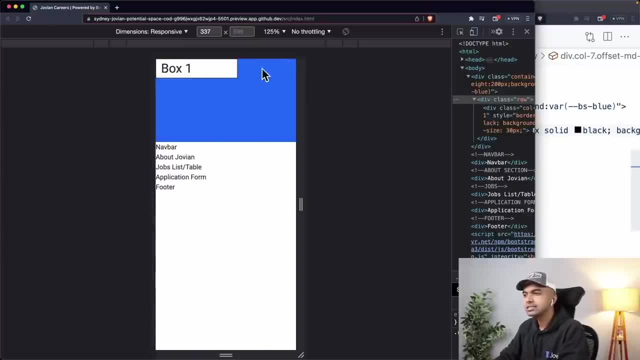 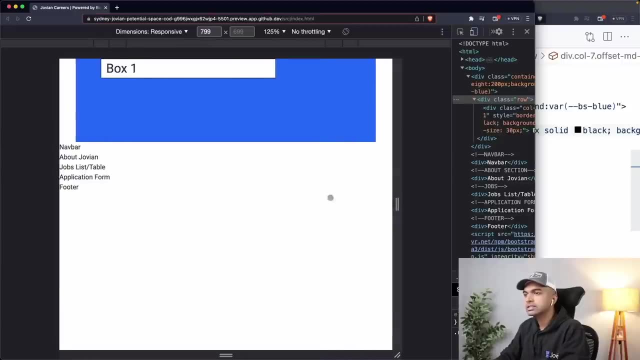 The column. it shows up right from the left edge and maybe there's something else I want to put here. But as soon as I cross 768 pixels, you'll notice here, as soon as I cross 768 pixels, this offset gets added. 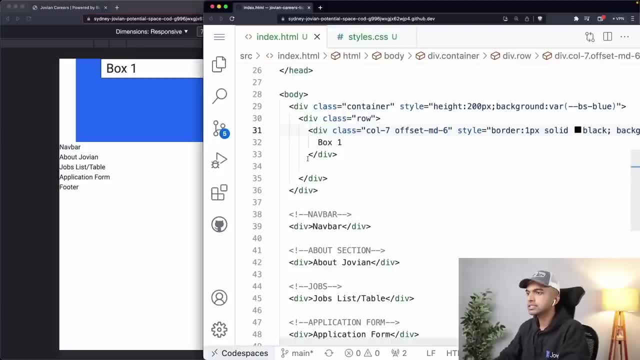 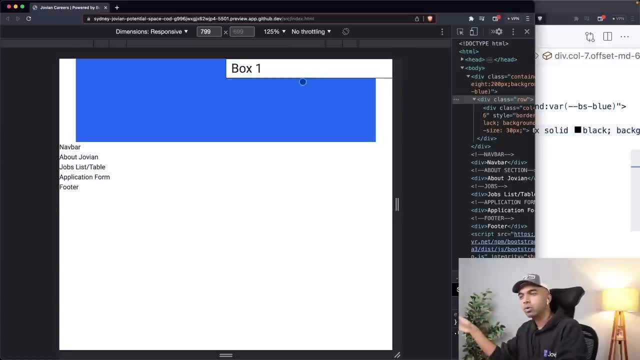 Okay, And I can control this offset. Maybe I want this to be offset six, in which case it is going out. now offset has this property that if you set too high offset, it's simply going to go out of the of the. 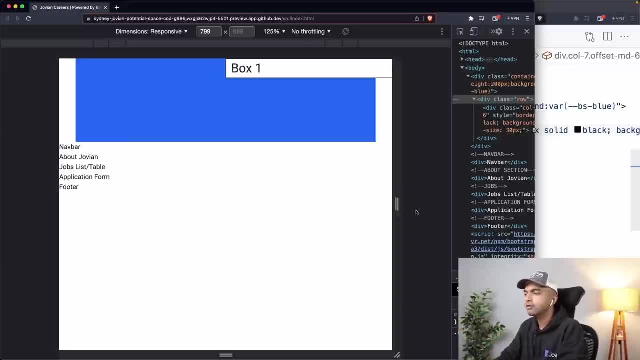 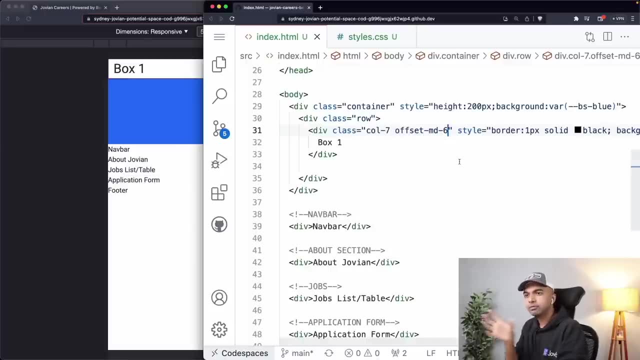 rope, It's not going to go into the next row because that doesn't really make sense for an offset. So yeah, So keep that in mind, that if you don't actually need to create a column, you just need to maybe shift a column a little bit. 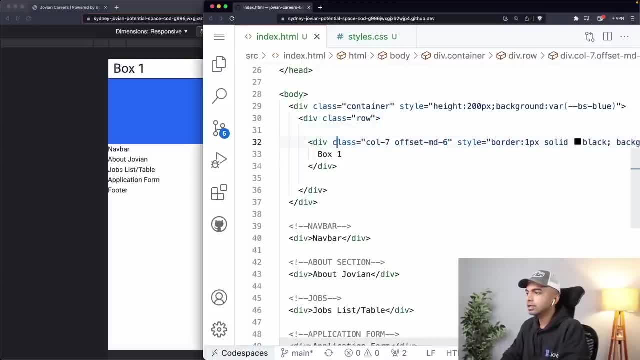 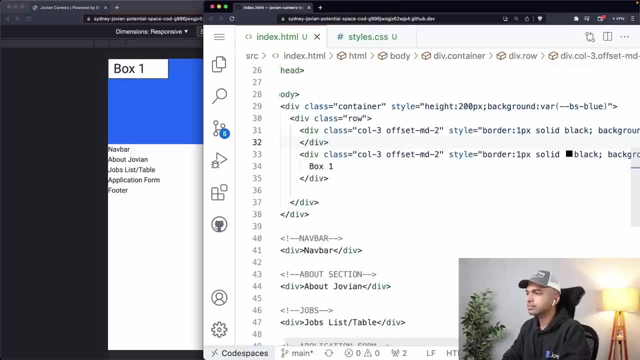 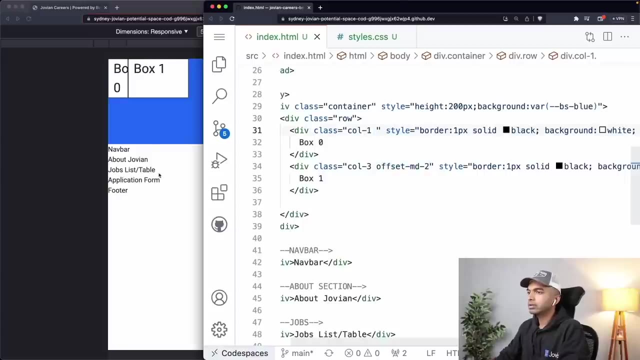 You can offset And of course you can combine things here as well. So you can do something like: maybe this is three columns with an offset of two, And above this you have another box. So this is box zero and maybe this is one column. 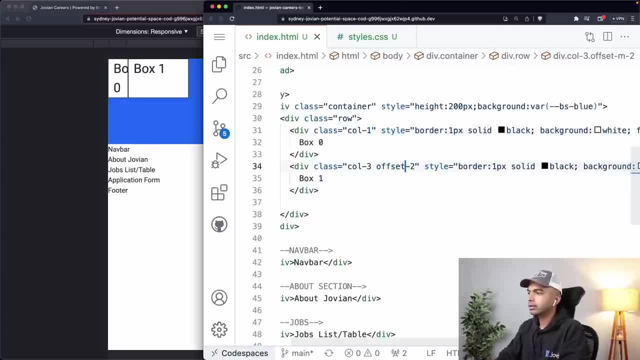 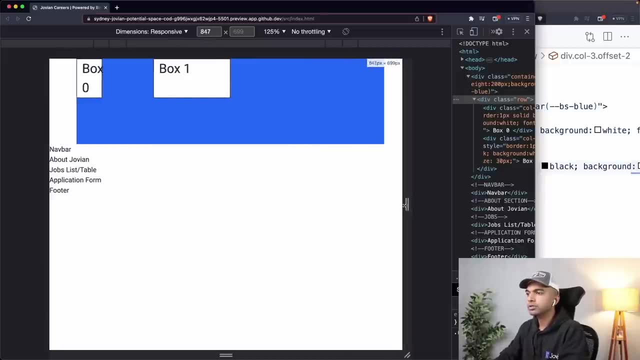 Yeah, So you could have something like this: You have this one column box over here, then you have a three column offset, and then you have a three column box over here. Okay, So you can create all sorts of interesting layouts using offsets. 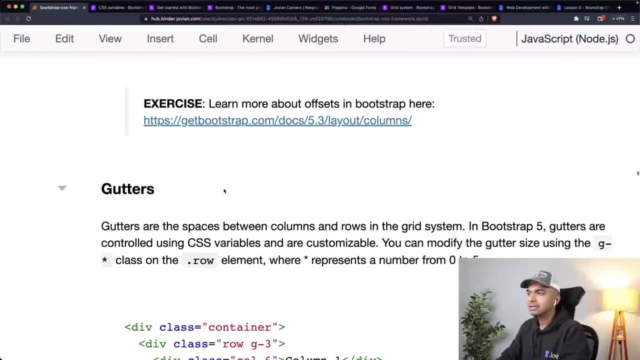 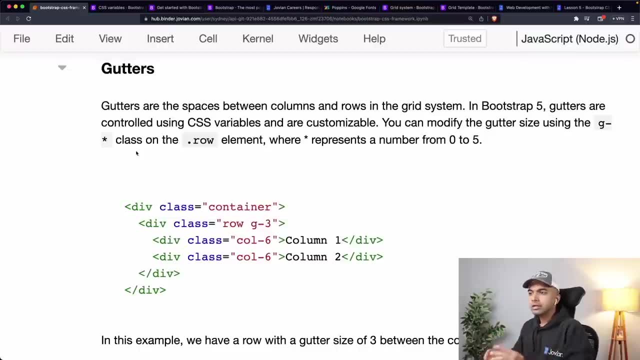 So that is all about offsets In The bootstrap grid system. Next, I want to talk about something called gutters. Now, in the grid system you can you have 12 columns, but those columns do not have to essentially necessarily stick together to each other. 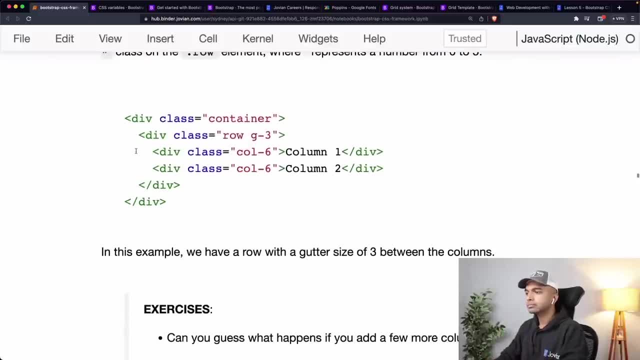 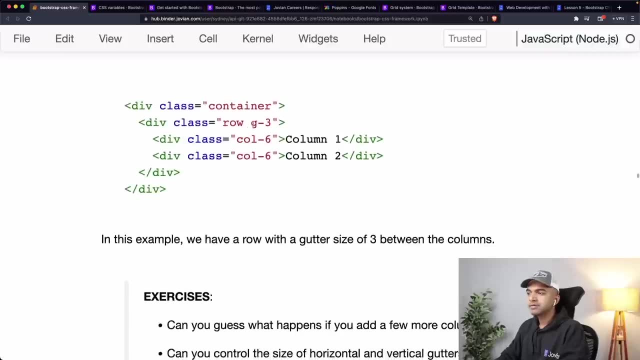 You can have a gap between those columns And you can specify gaps between those columns using the gutter or the G or the G class, So you can specify it at the row level. You can simply say that you're when you're creating a rule, you want the gutter to be. 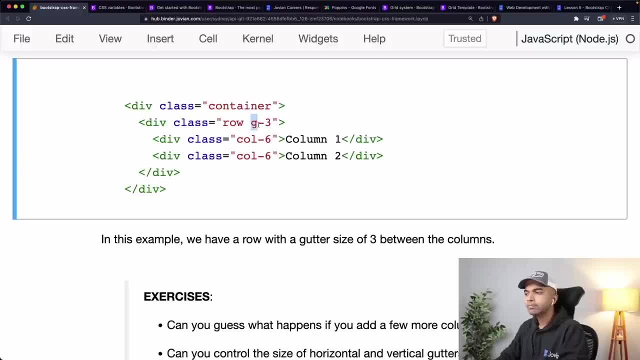 you want the G class? Okay. You want the gutter to be of a certain size? Okay, And the there are sizes. the sizes go from zero to five, and it's not zero to five pixels. You can actually check, inspect and check. 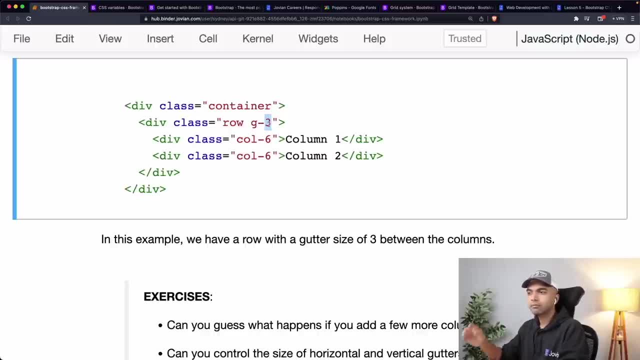 I believe it's zero time, I believe it's some multiples of four or something like that. So a gutter of three would essentially result in three fours about 12 pixels, or there is some kind of a ratio that that it actually ties into. there is some responsive layout. 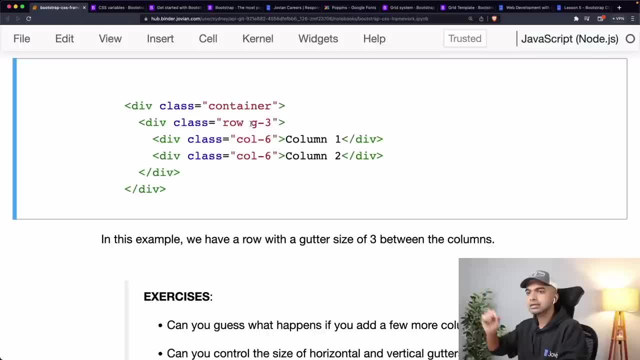 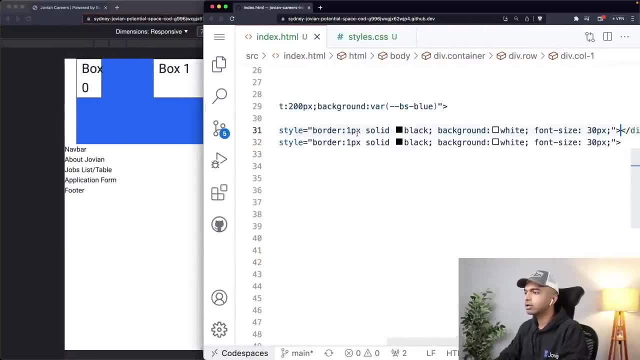 that it handles. but just think of the gutter sizes as a sort of a scale, Sort of a scale of zero to five that you can modify things for. Okay, So let us come back here and let us maybe revert to the columns that we had. 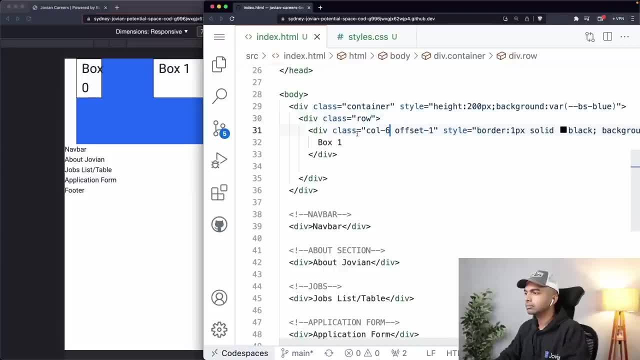 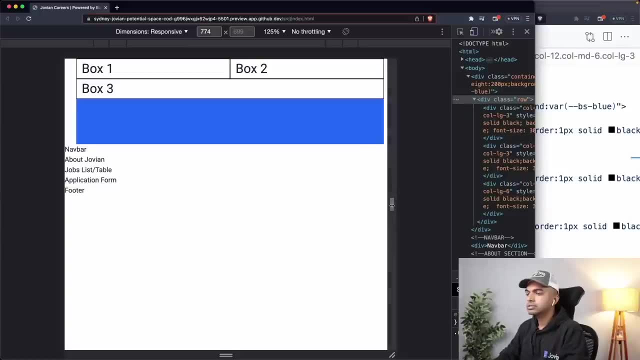 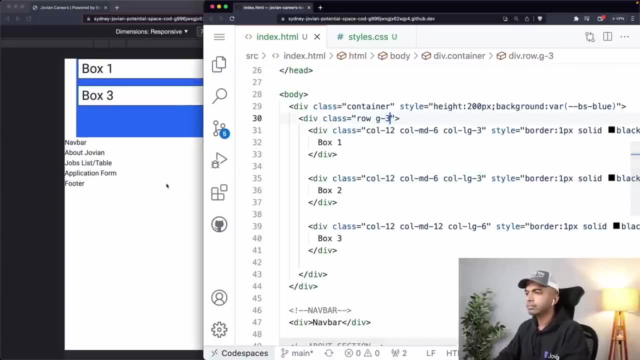 So we had three columns here. Yeah, So we have three columns here and all these three columns you can see show up like this And there's a sort of a responsive design and play here. already Now, if I just add G3, you can see that some content or some. 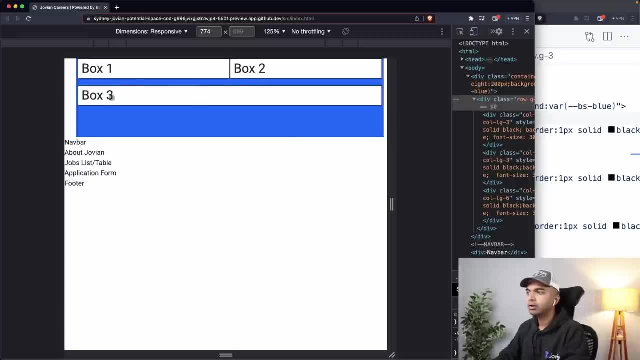 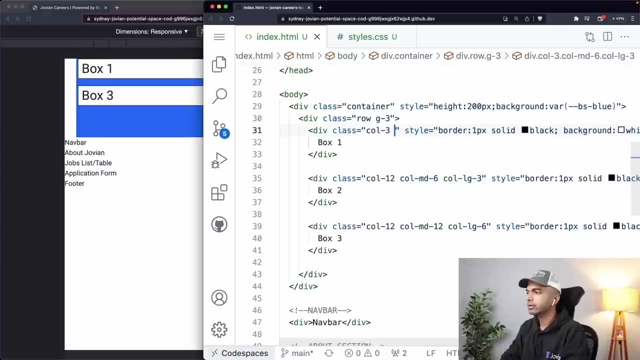 Splitting, Splitting. Some space has been added on the left and right And also between these columns, And for now let me just make these very simple columns. So I'm just going to make it call three. Each of these is going to be a call for yep. 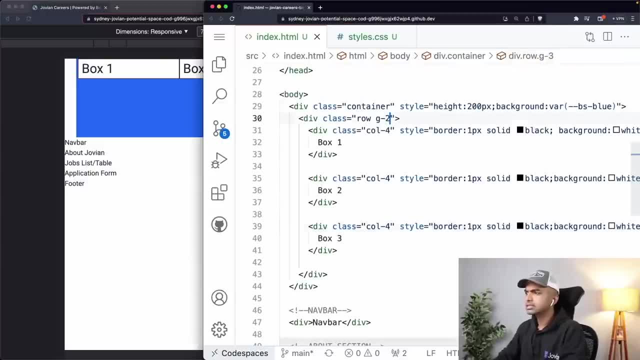 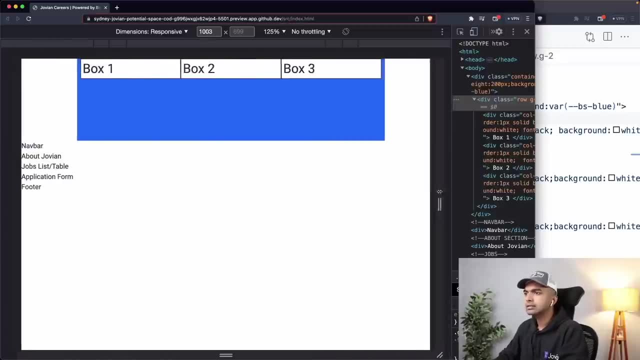 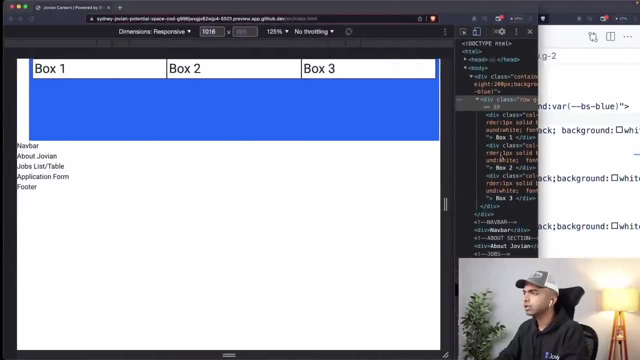 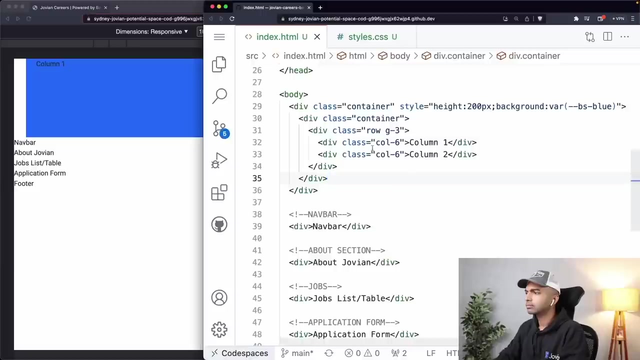 So you have a call for, and maybe G3 doesn't seem to be working. Okay, It is. Yeah, So this is, and as we increase the space, you will see that the gutter should increase. Let's see. Well, this doesn't seem to be doing the job, probably because of the let's add a border. 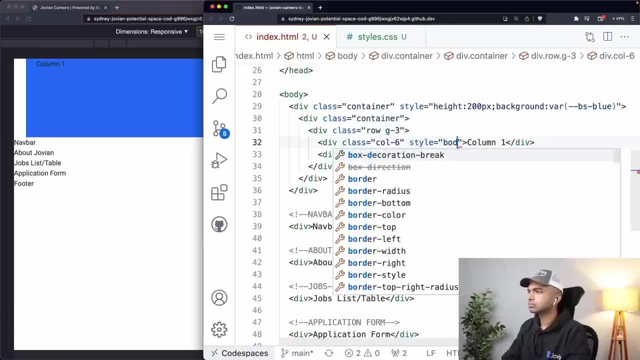 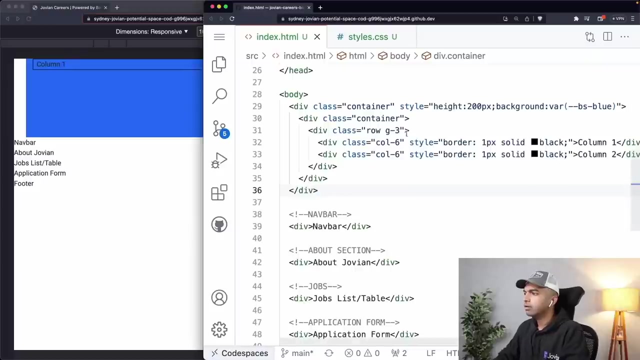 to this. Okay, Okay, Okay, Okay. So let's take a look at this so you can see that there is some gap here and there is some gap here. Now, if we remove this gutter, you can see that some of that gap disappears. 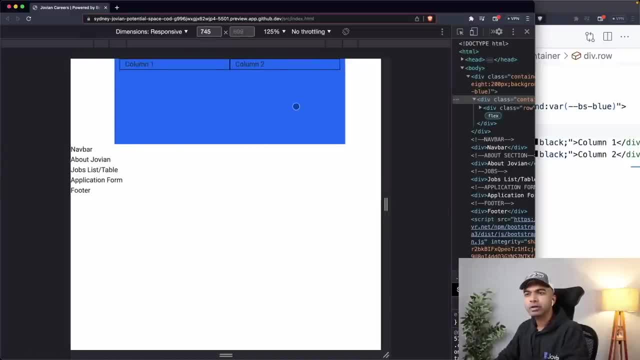 Now that gap should also show up between columns. I am not a hundred percent sure why it's not showing up right now. Maybe it's I, maybe that that gap is actually getting as going to get added inside the border. That's why we're not seeing it. 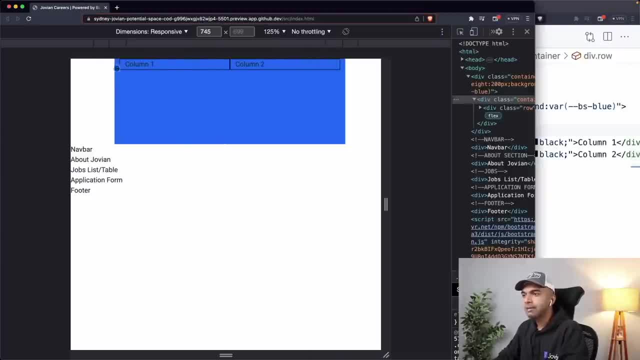 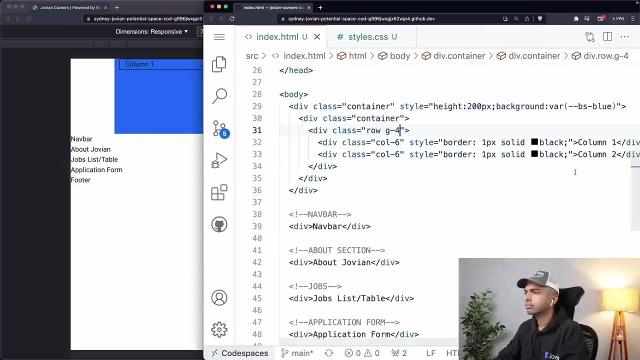 But yeah, So what the gutter does is it adds gaps on the left, right And between your columns, right, So you can check maybe G4, or let's just try GX4 and GX4.. Okay, Okay, Okay, Okay. 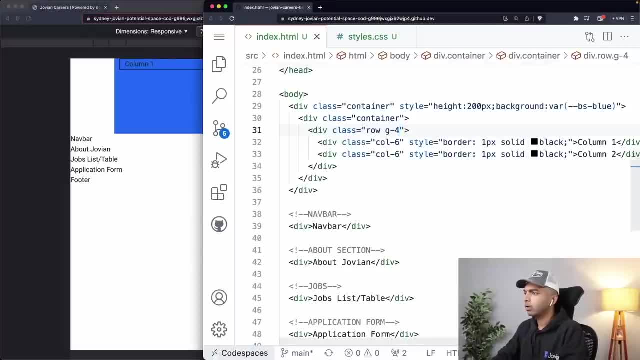 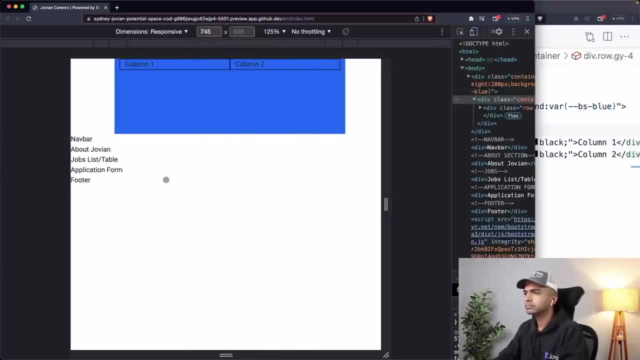 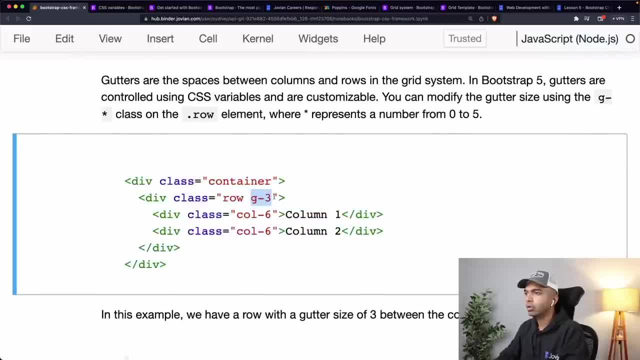 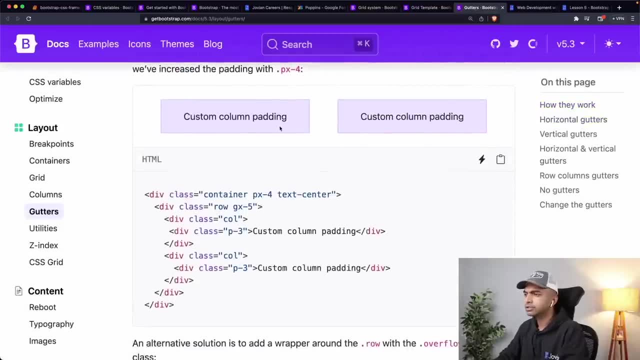 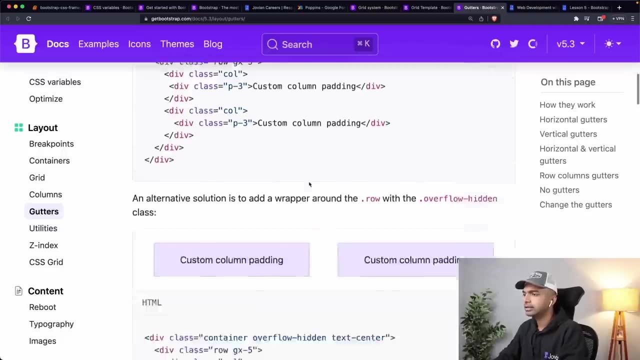 then you can simply say the God On the row variable. Okay, So you can check out the documentation for gutters here. This is this is exactly what it should look like. So there should be some column, There should a space here, some space here and some space here on the right. 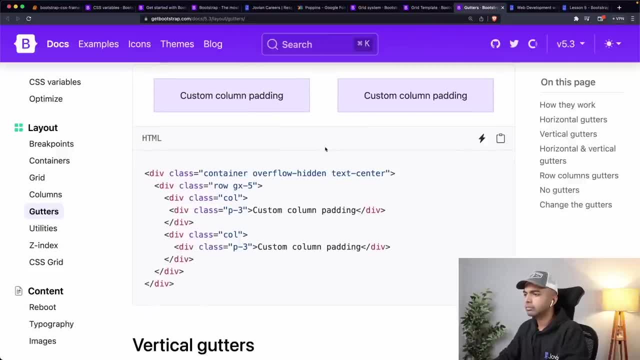 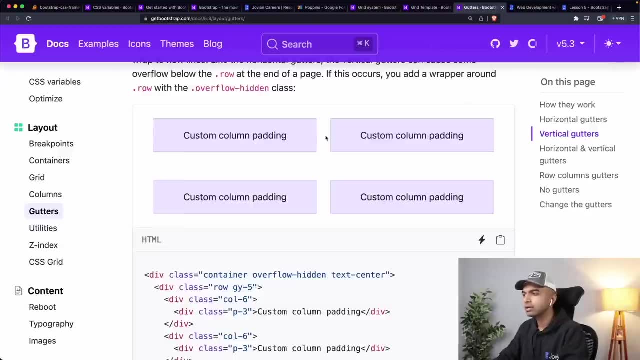 And similarly here you can see that there is a gutter on the left and right And that gutter can also be changed, customized, on the left, right and bottom as well, So you can have some spacing between the columns, You can have some spacing between the rows when things overflow into the next line. 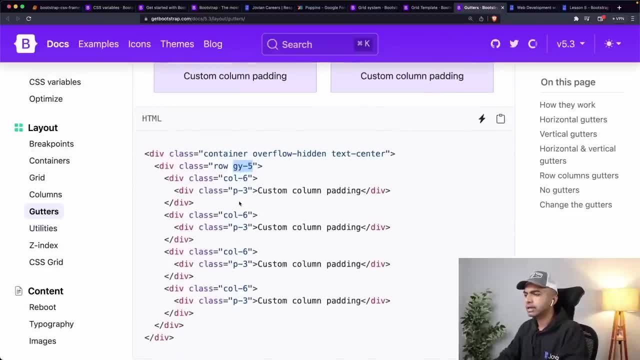 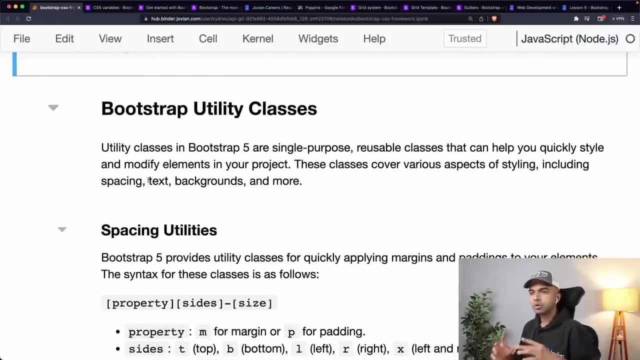 And that is being set here. You can see using G by five and so on. Okay, So that is all about how you use the bootstrap grid system. So the key things for you to keep in mind are: always use a container, And the three types of container are a container that is always kind of centered and restricted. 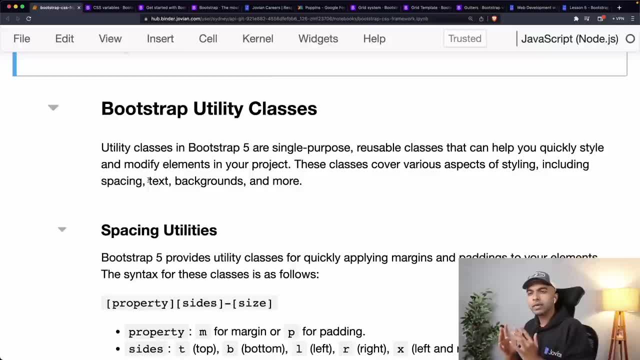 And then a container that is completely fluid, that always takes up the full width of the page, and a container that takes up a full width up to a certain breakpoint And from that breakpoint it remains centered on the page. Okay, So just use bootstrap containers. 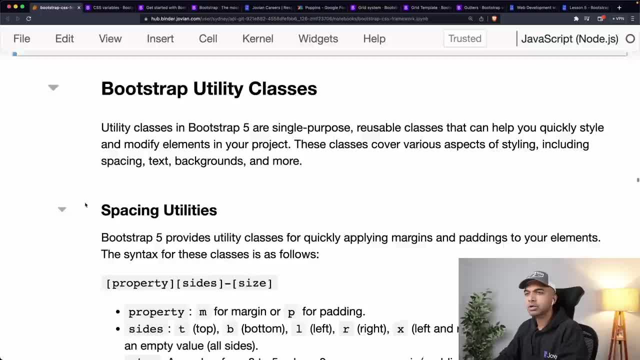 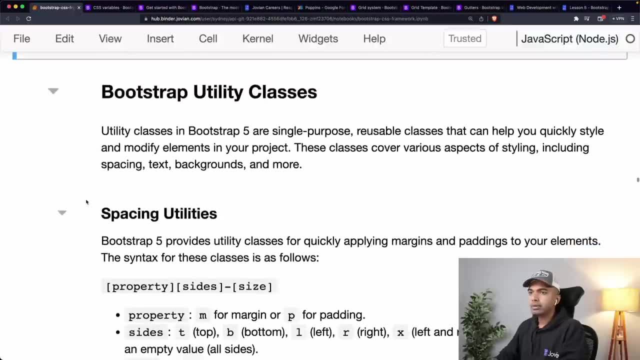 You don't have to create your own containers or add your own breakpoints or maximum widths. Generally speaking, your bootstrap container should do the job for you. Okay Now, apart from containers, you have rows and columns, so you can create a row and then. 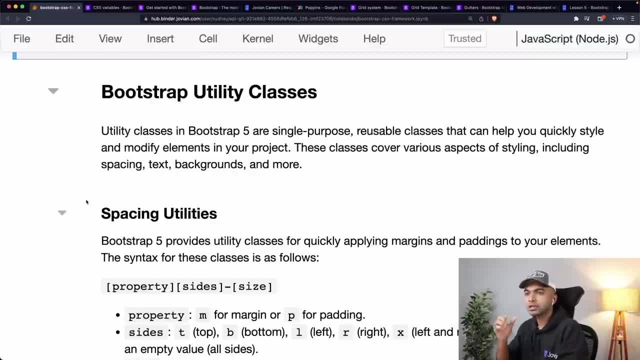 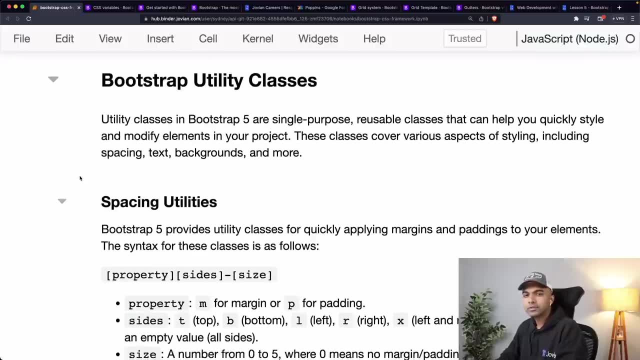 you can put a bunch of boxes in a row and then you can specify their widths using the 12 column grid system, And you can change the widths based on certain breakpoints. You can also then use offsets, and you can also specify specific gutters and based on. 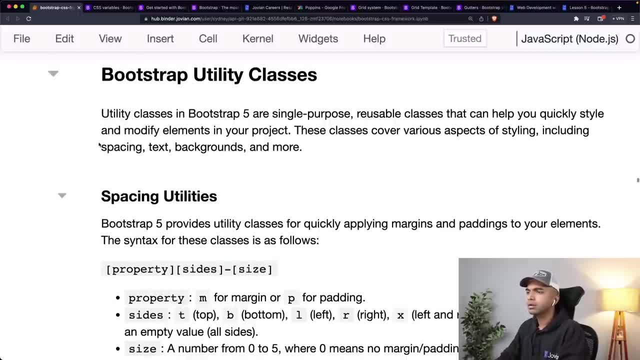 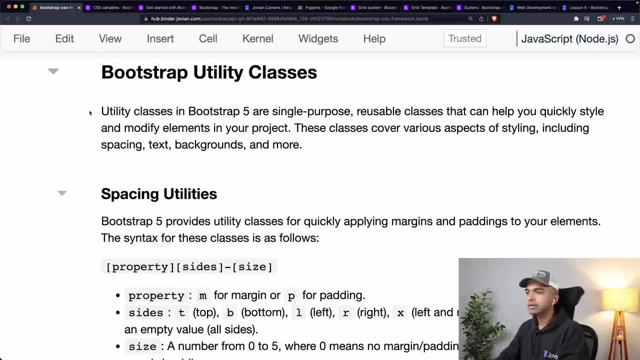 the gap that you need between your columns. Okay, Now, next thing, I want to talk about Bootstrap utility classes, because this is also something that we're going to use when we start building our websites. So utility classes in bootstrap are single purpose, reusable classes that can help you. 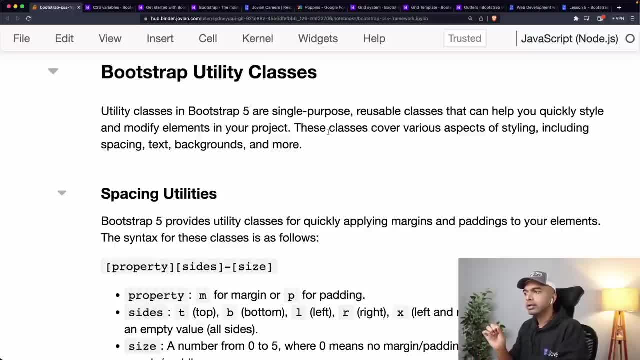 quickly style and modify elements in your project, And they include various aspects of styling, such as spacing text, backgrounds, etc. The key idea here is, for a single line of CSS property that you might want to put in the CSS file, you can simply include a utility file, utility class that's going to do the 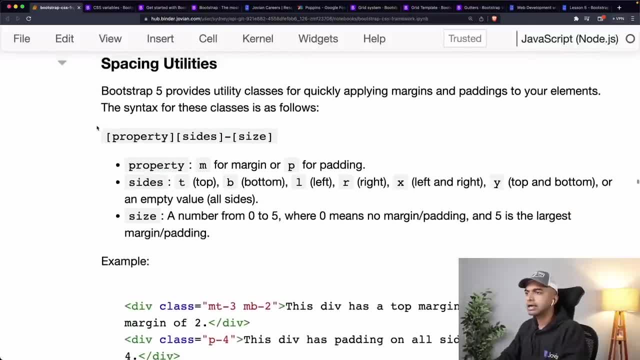 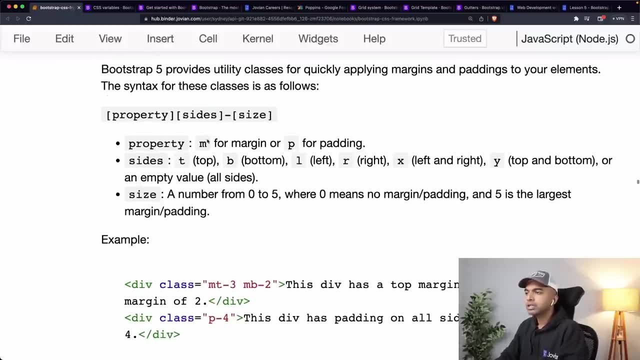 job for you. So here are a few utility classes that we're going to look at. the first is spacing related utilities. Spacing simply means margins and paddings, So bootstrap provides a bunch of classes like this, So you can say: empty hyphen three. 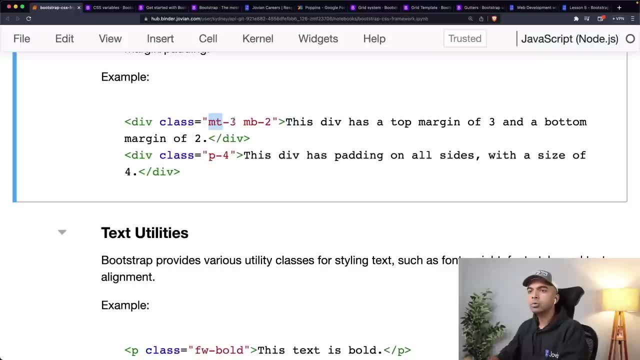 And what that does is it says margin top should be set to three. And again, this is not three pixels, this is just on a scale of zero to five. this is a certain five is a very high pad margin. zero is zero margin, so it is just somewhere in. 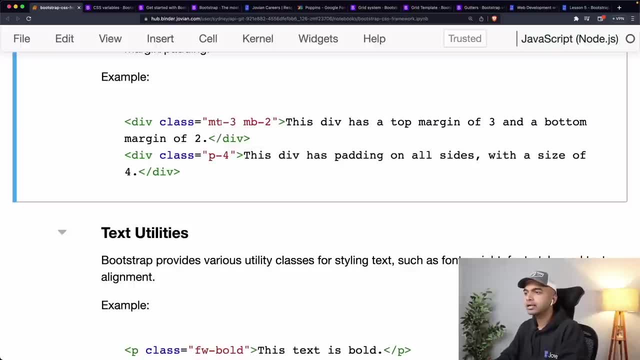 between, So you can specify what the actual value is by inspecting it in your browser. And similarly, you can say mt three or you can say mb two. okay, so T includes a, T means top, B means bottom. So just using these few characters, we've specified the margin top and margin bottom. 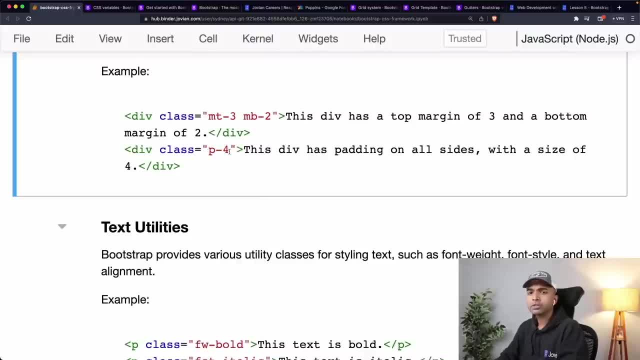 Or we could also do something like this. we could do P hyphen four, which means that you want a padding of four units, not four pixels, four units on all sides. Let's see what that actually means, So let's maybe go. 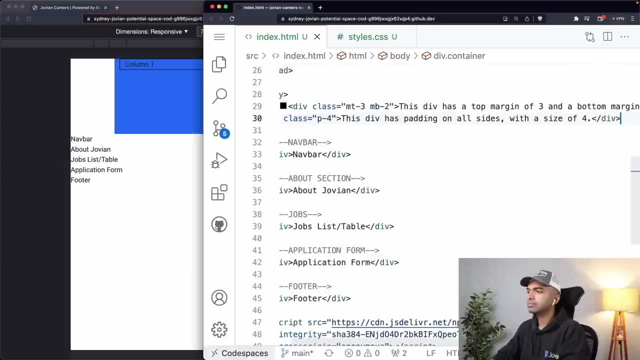 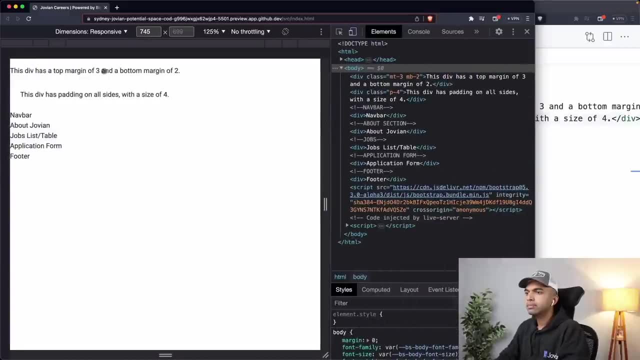 In here, get rid of this container over here and simply post these in. So you can see now this particular div that we have here. this div has a top margin of three. And what do we mean by three? Well, if we just look at the styles for this div, the computed styles, you will see that 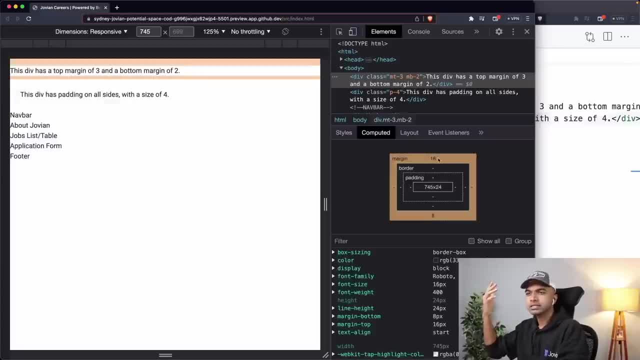 this div has a margin of 16.. So three simply means maybe about 16.. And this div has a bottom margin of two, So that is eight. So I believe it works. One is four and two is eight, and three is 16 and four is 32, and so on. 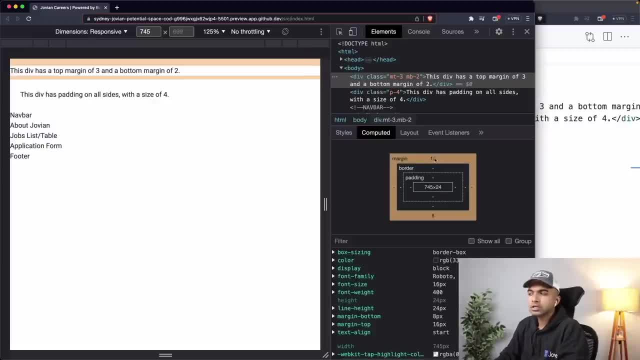 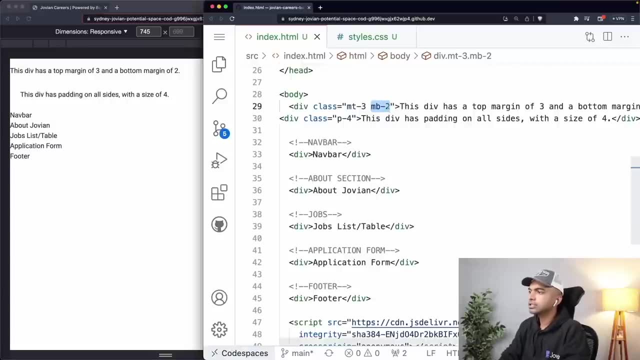 So yeah, so mt three means a margin of 16 pixels at the top And mb two means a margin of four, eight pixels, And you can go ahead and change this. You can change this to maybe mb five and see what that changes it to. 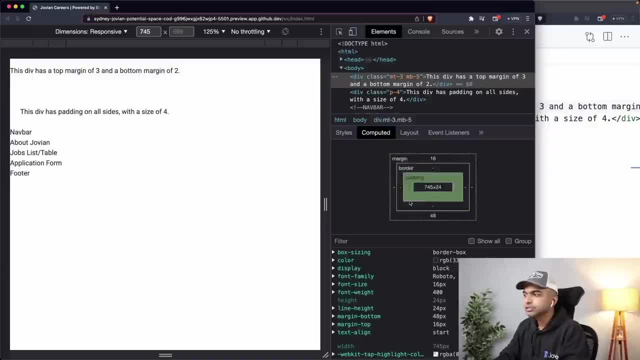 Now the margin becomes 48.. All right, So you can always check what these margins are. And let's check this div. So this div does not have margins. But this div has padding, So it has a padding of four pixels all around it, or a padding of 24 pixels all around it. 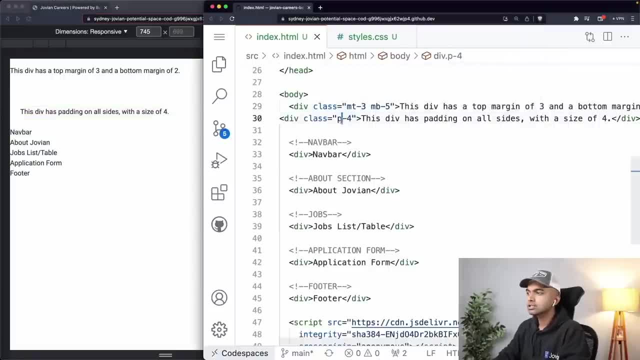 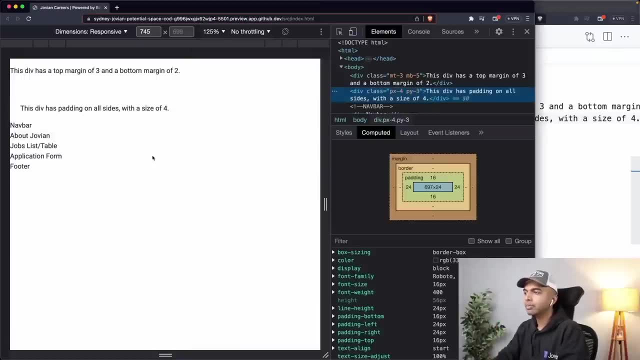 So p4 simply adds 24 pixels on all sides. I could also do px four and py three in case I wanted to. just x direction is left and right and y direction is top and bottom. Now you can see that top and bottom, py three applies a padding of 16 pixels and left and 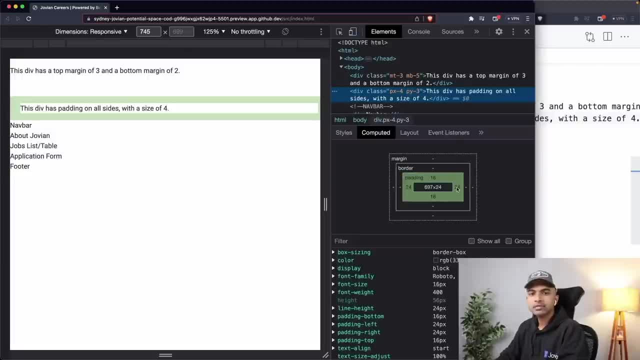 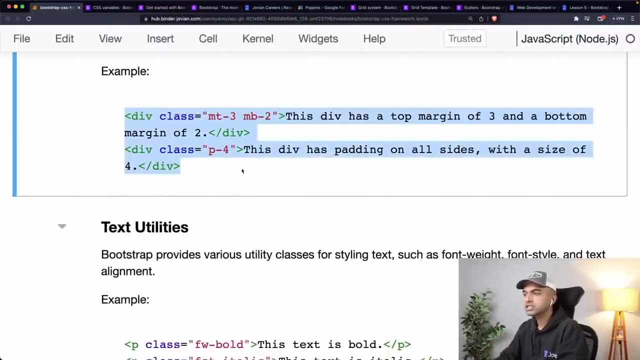 right py four applies. our px four applies a padding of 24 pixels, So this div has padding. So this is how you can quickly apply paddings, and they've already set some some default values so that the spacing doesn't look very off. So always just try out- maybe mt one, mt two, mt three- and see which one works best for. 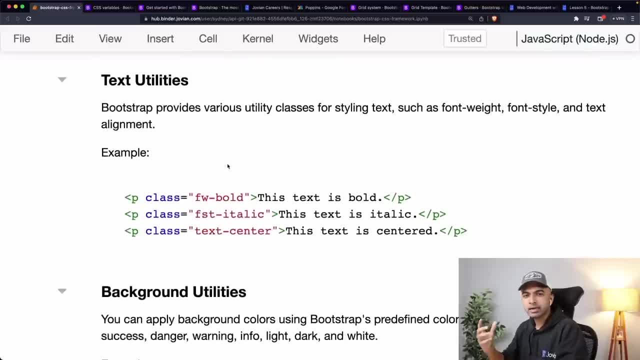 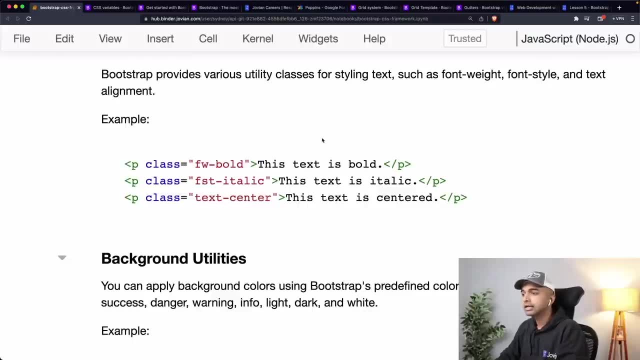 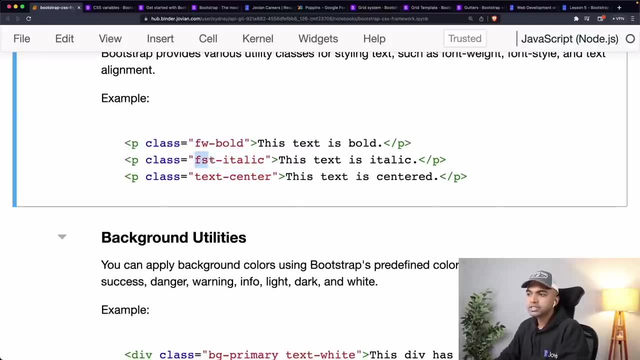 the layout. Okay, so those are the spacing related utilities. Apart from that, we can also use utility classes for styling text. for example, you maybe want to send us some text, or maybe you want to make these, make it italic, or so FST stands. 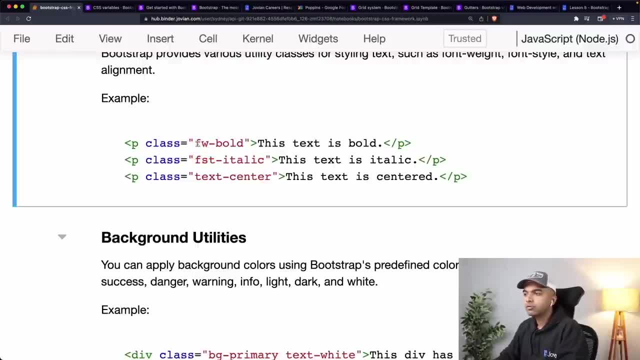 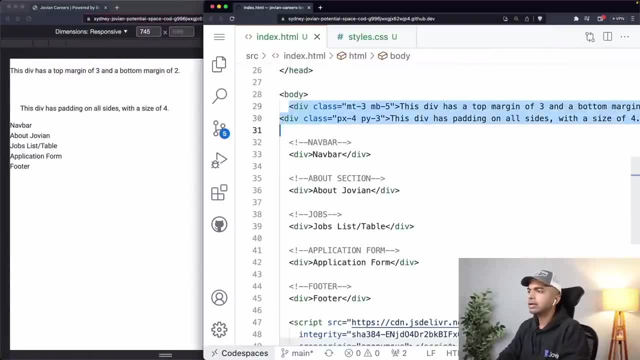 for font style, Or maybe you want to change the font weight, you want to change the font weight to bold, So all of those things are something again you can do using utility classes. So I can come back in here And I can just drop this in. 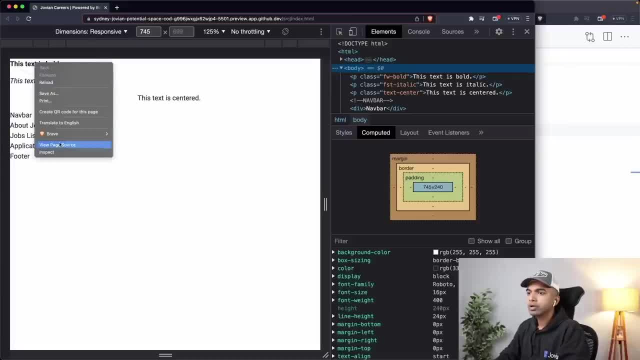 And you should see that this text is now bold because it has the class FW bold. And, by the way, if you're ever curious, what styles does a particular class actually apply, you can come into the inspect tools and you can check the styles tab and in the styles, 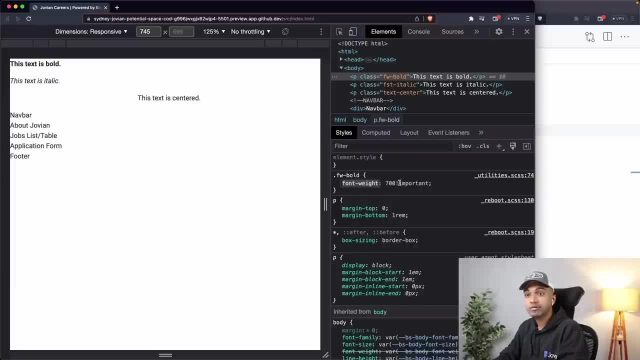 tab. This FW bold applies the font weight of 700. Okay, so that's what it actually does. So there's a very deep level of CSS inspection that you can do whenever you're looking at a website, or maybe you just use some bootstrap class and you want to know what exactly it. 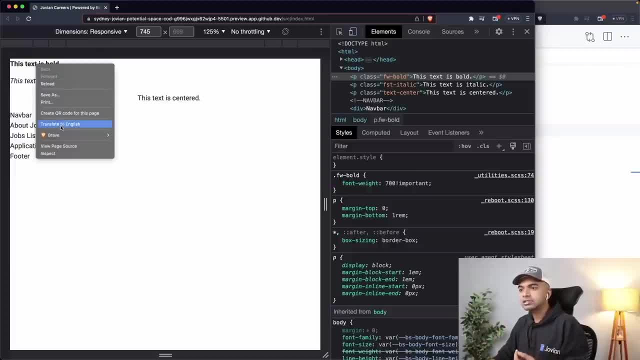 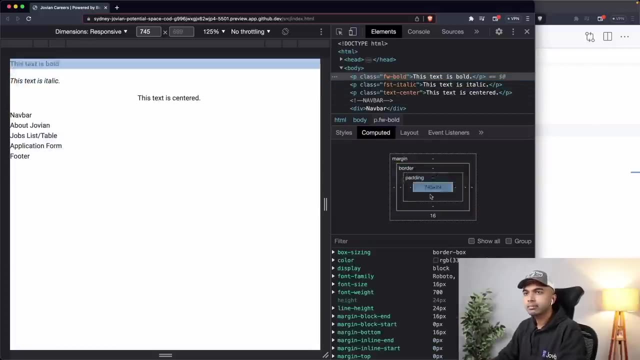 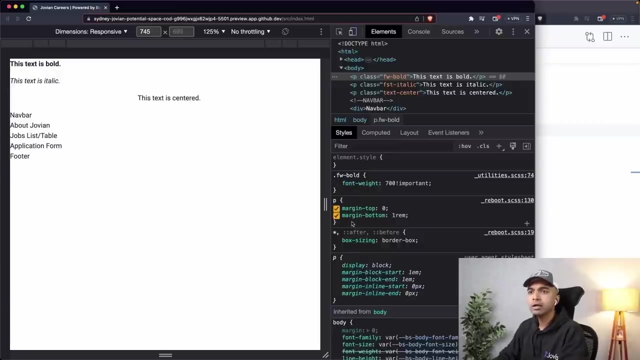 does Just right click on the text, just click inspect. Oops, yeah, just click inspect, Just click inspect, And then you can either check the layout here using in the computer tab, or you can go into the style style styles tab and see the exact styles that have been applied for each of. 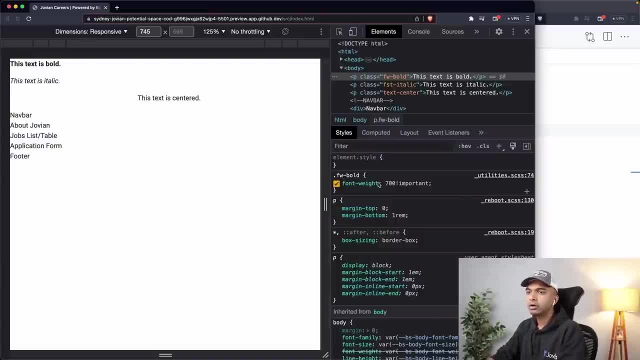 the selectors that apply to this particular file, okay, or to this particular element And FW. bold is clearly coming from bootstrap and it sets a font weight to bold. Let's check this one: this FST italic, this text: this sets a font style to italic. 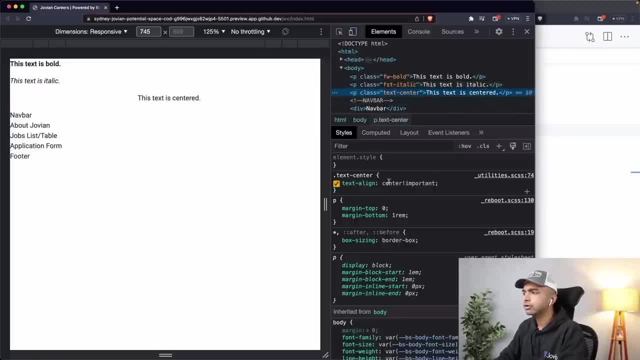 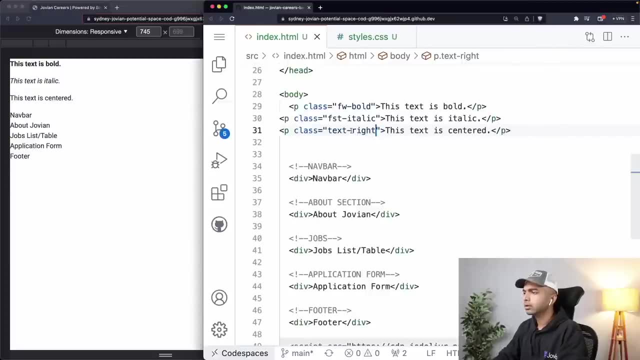 And then we have text centered. This is We're simply going to center the text. Of course, you could also do text right or something like that, And that is going to put the text on the right. Maybe it's text aligned right. 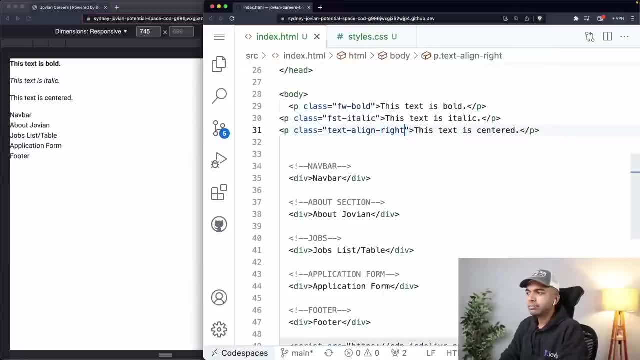 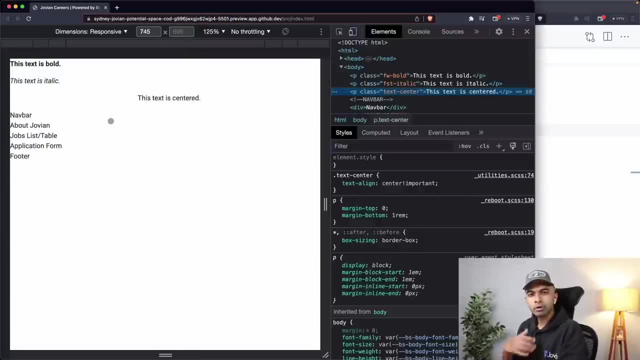 Okay, I don't know. So, yeah, maybe there's a way to align the text to the right. I would just probably look it up in the documentation. So how do you know these? how do you know what utility classes are available? 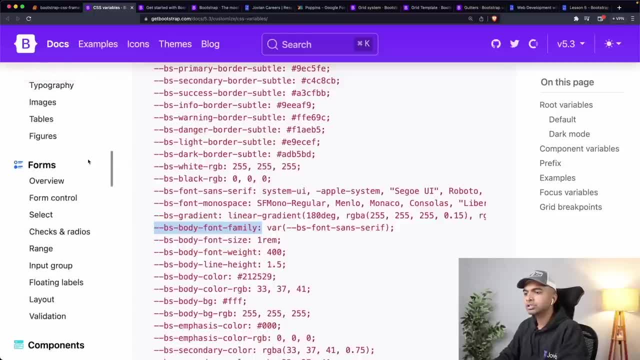 Well, you just have to check the documentation. If you check the documentation of bootstrap, you can see that There is a section called utilities and then there are various utilities for text, display, flex, et cetera. So we were looking at text and you can see that there is text alignment. 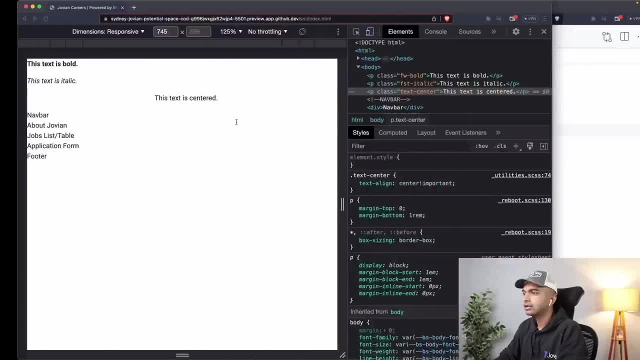 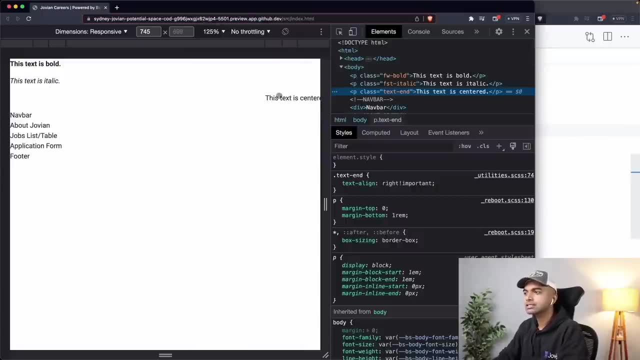 So you have- Okay, You have- text start and text end. So if you want to align something right, you have to say text end. and this is because it supports the right to left layouts as well, And you can see that now Texas moved to the end. 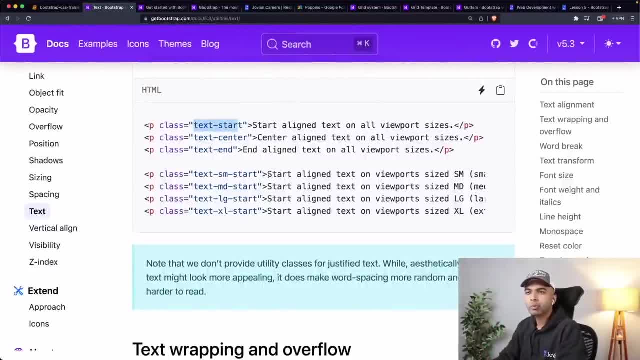 So I would just keep the utility section of bootstrap open and look it up. How is it Better? What classes in your CSS file? Because by using a utility class, you are co-locating the style with the HTML, So at a glance it's going to be very easy for a developer or just for you to be able. 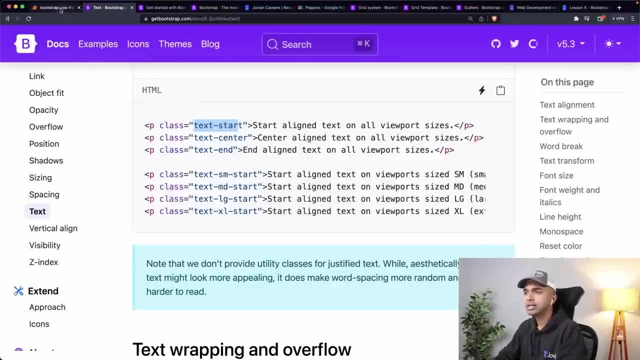 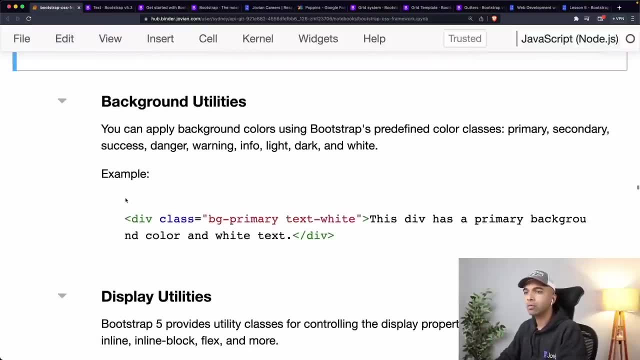 to identify what are the styles that are getting applied to a particular HTML element. Okay, So utility classes are great because they just bring the styles into the HTML and help you get a clear picture of what the what the element is going to look like. 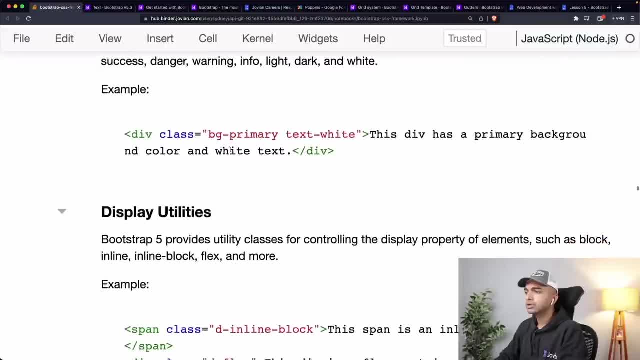 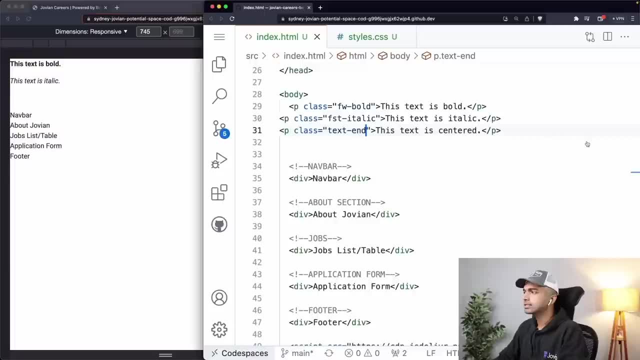 Okay, Okay, Okay. So you could do something like this. You could, let's say, set the background color to the primary color, which is the blue that we have set. So let's create this div over here. Let's get rid of these text utility classes. 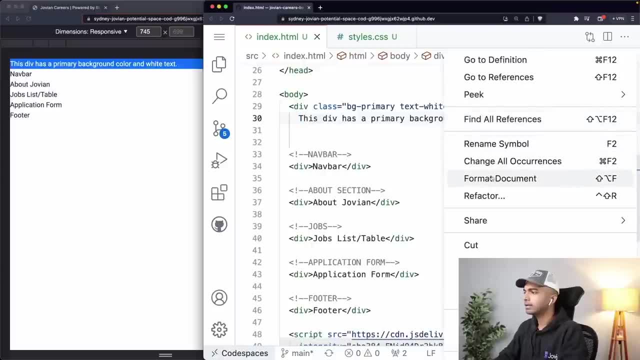 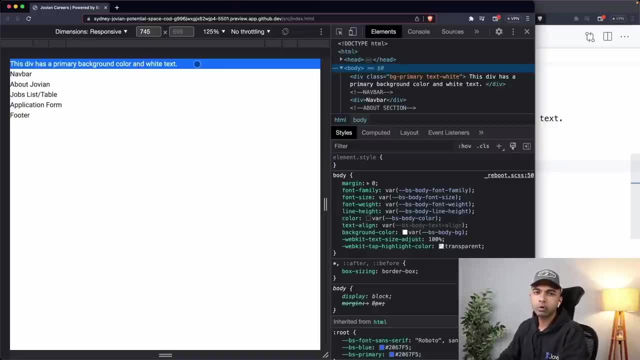 And this is a particular div. Let's format that. Yeah, So you can see that this div has a primary background color, which is the blue color that we've set, and it has the color of the text: white. So you can say text white. that is going to simply change the color of the text. 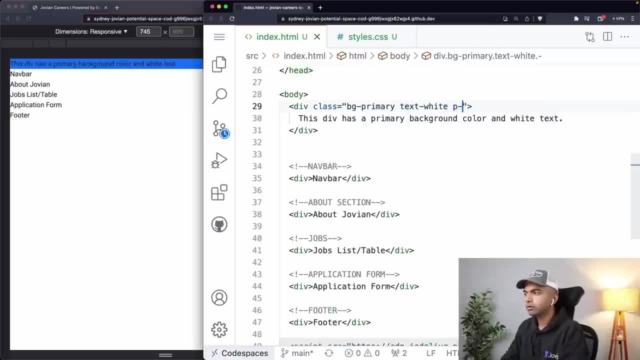 And I could also do something like P4. Let's say, if I wanted to add some padding to it and I could also add borders and things like that. So there are lots of utility classes available that you can apply here. There are also display related utilities. 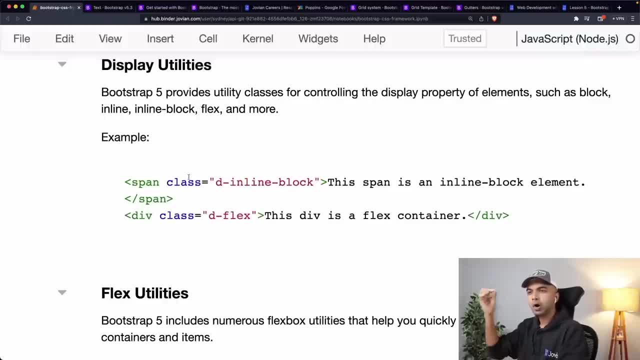 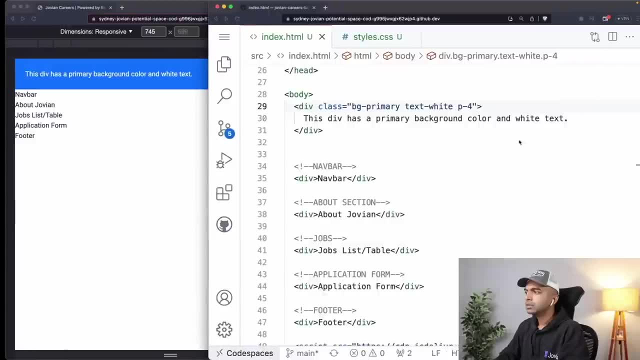 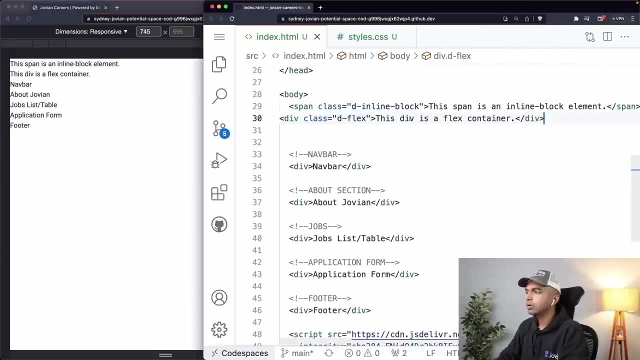 So let's say you want to change the display property. Remember, you can have block, flex, inline, all of those things. You can do all of that using display properties as well. So let's look at an example. Okay, So now we've created the span and we've set its display to inline block using D hyphen. 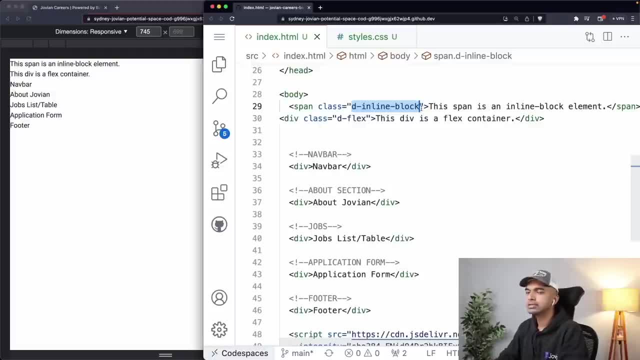 inline, hyphen block. So the shortcut or the shorthand for the display utilities D and hyphen inline, if you wanted to show it inline, or hyphen block, if you wanted to show it, block within inline. So all of these are different meanings. 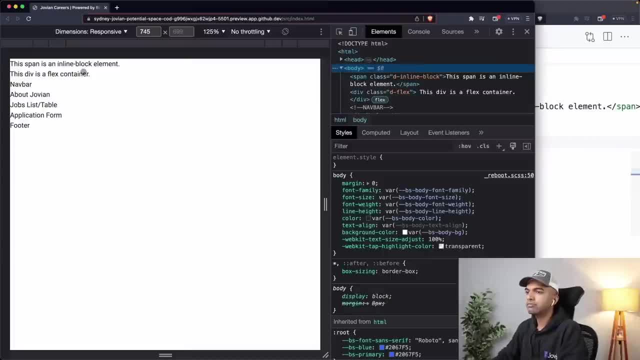 This is going to turn it into a flex container And again, you can verify. you can just go in here and click inspect. You can check that this is actually. this has the display type flex. You can verify that it actually has the display type flex. 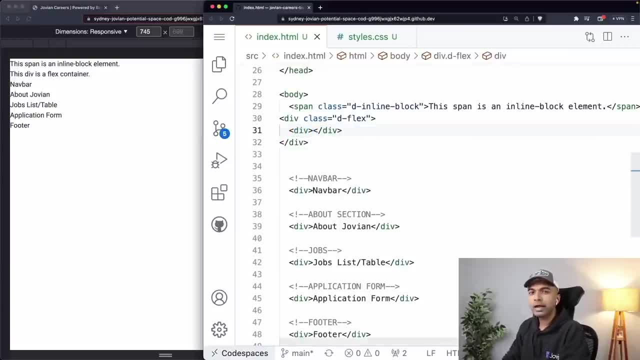 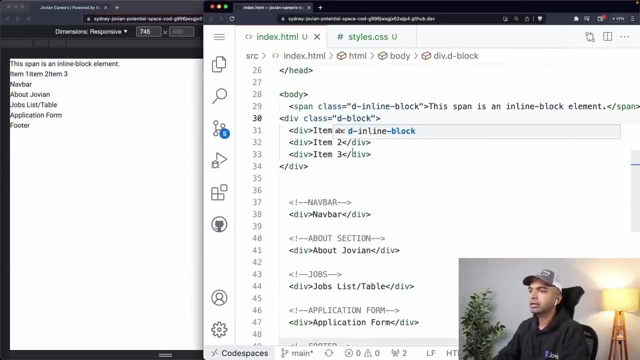 Okay, So this actually has a display type flex by putting a bunch of items inside it. So let's say, let me put item one, item two, item three. you can see that they show up in a row. Of course, if this was not flex but if it was block, then item one, item two, item three. 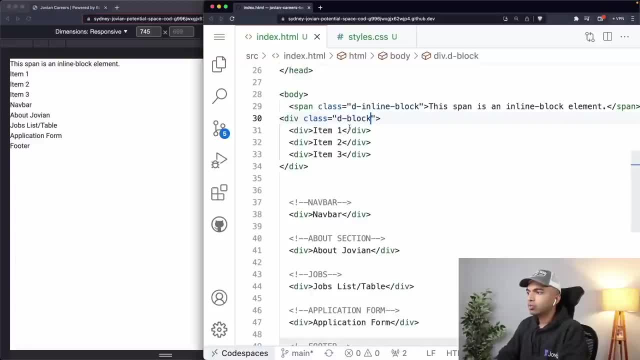 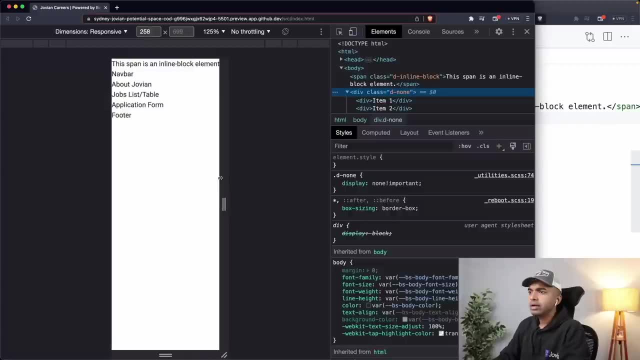 would show up one below the other. Okay, But- and I could also have set it to D- none. So I could have done something like this- that this is just simply not visible. And here's one trick: Okay, Let's say you want to make something visible for a particular size, for a particular break. 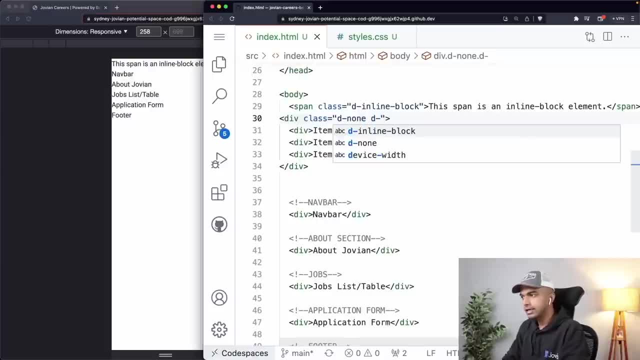 point. So you can say D none, and then you can say D MD block, or let's maybe say D SM block And let's say D MD flex, Okay. So what we're saying here is: I don't want this div to show up by default. 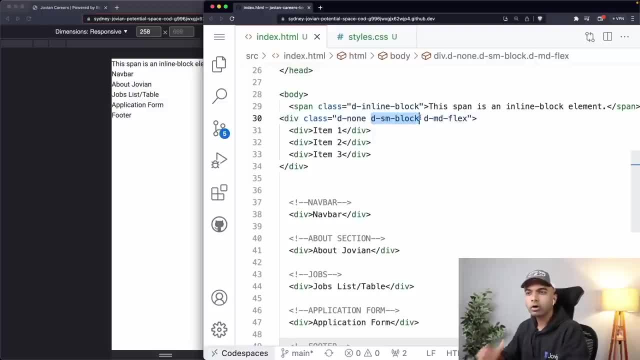 I want this div to show up as block on SM and higher, which means 576 pixels, Okay, And then on 768 pixels and higher, I want it to show up as a flex div, which means it's items are going to show up in a row. 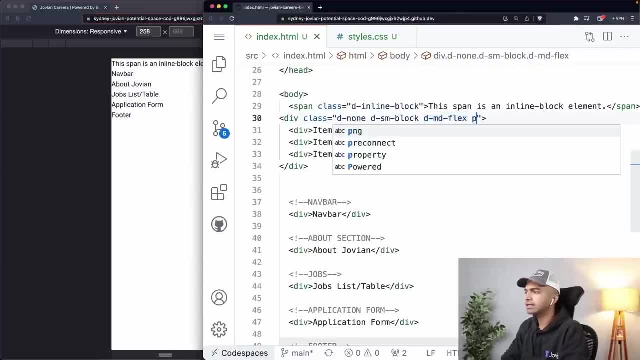 Okay, So here this, and let's just give it a little bit of padding as well. So let's give it P3 and let us give it BG blue, so that you can actually see what's happening here. Okay, So, right now that div is not showing up. item one, item two, item three: let's get rid of. 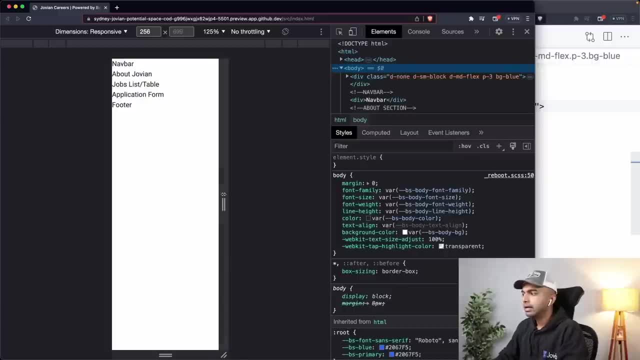 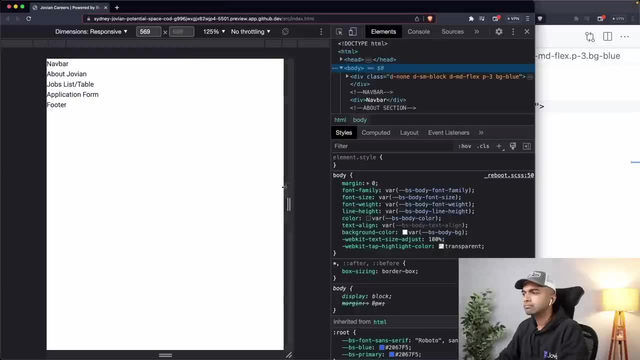 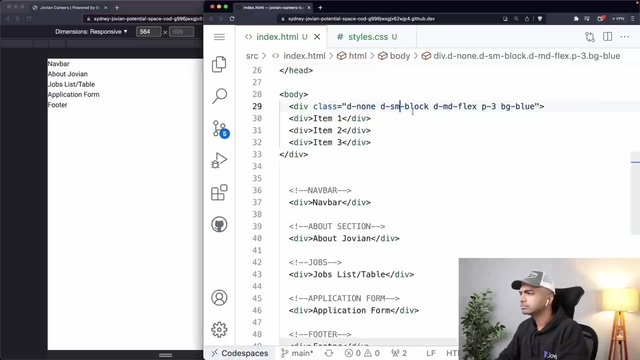 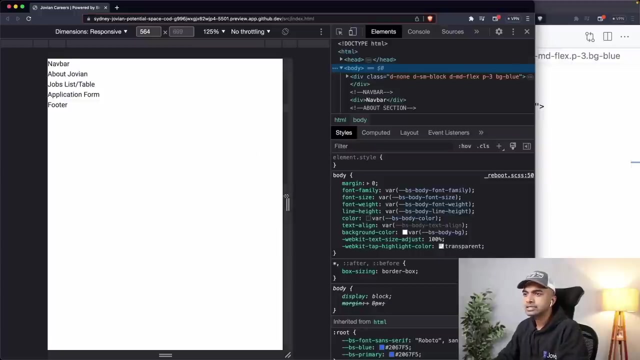 this upper span, Okay, Okay, So what if I just increase it slightly? okay, I guess D SM block did not actually work out here for some reason, I'm not sure why, but DSM block should also show up. but you can. 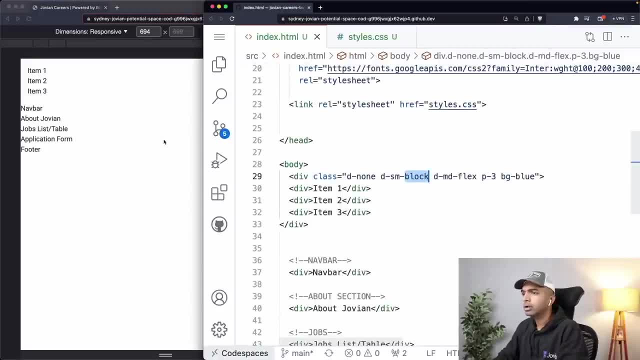 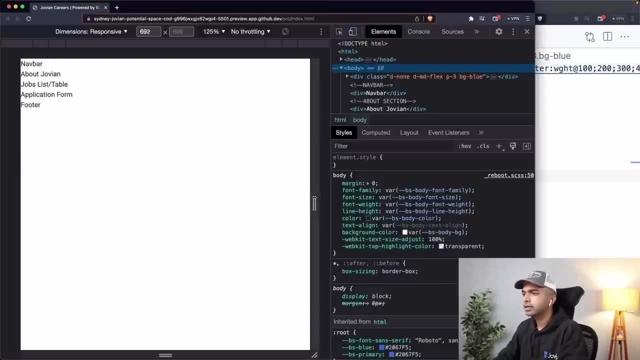 see here, when we set, when we set it to- let's just put it this way: Okay, That initially it's set to display none, And when we close, when we go to MD, we want it to show up as flex. 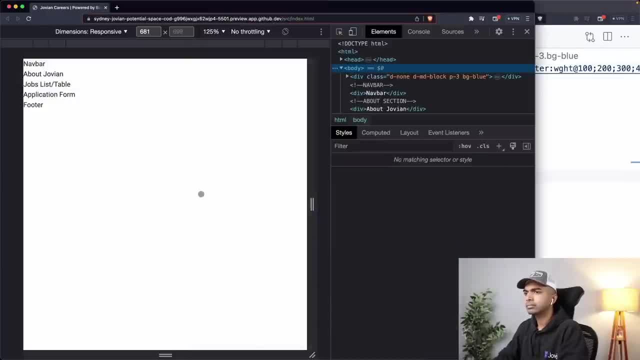 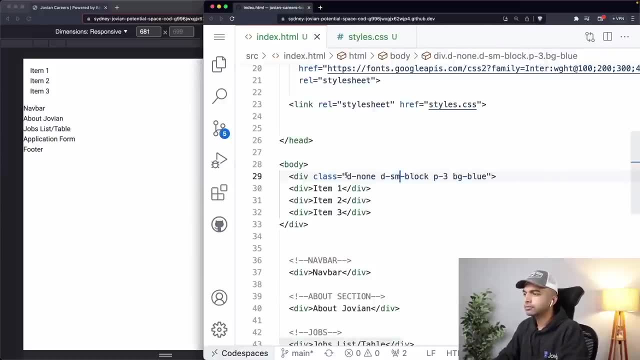 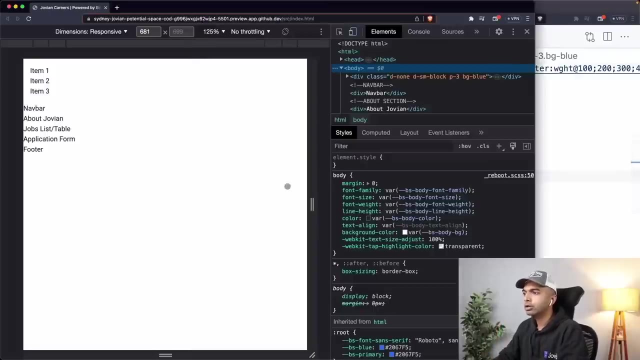 Yeah, Okay, Let's just look, let's just do this. So D none. So it is none by default And when we go into the SM layout, which is the small layout, is going to turn into block. So D none. 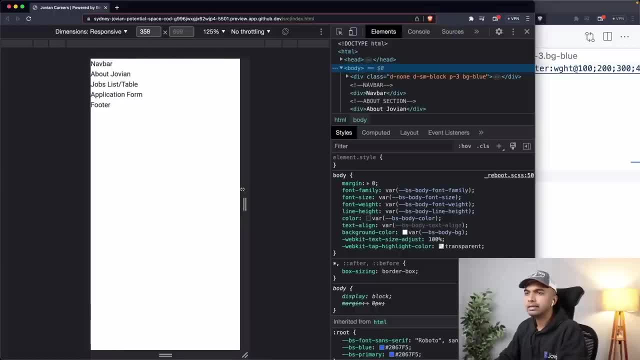 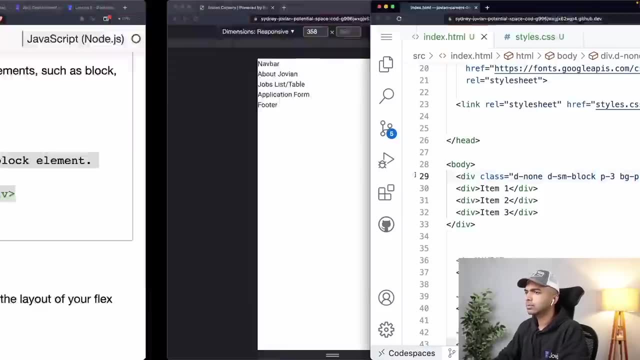 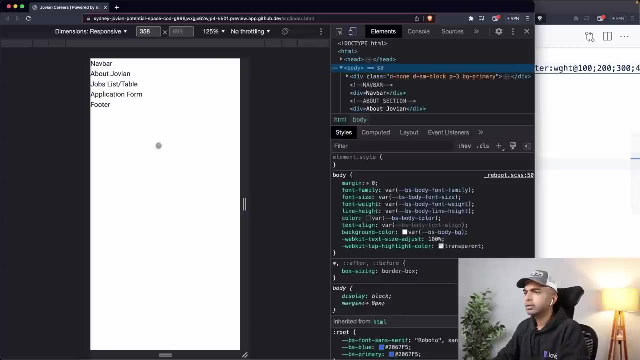 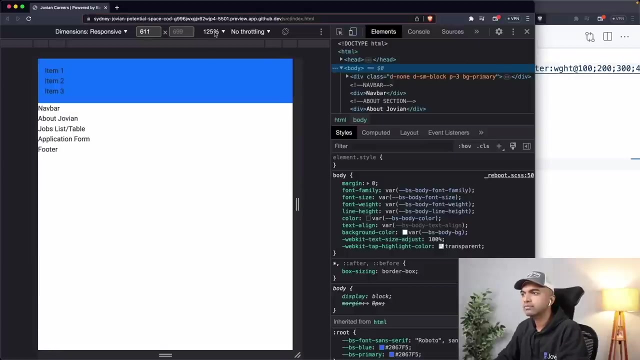 So you can see that below by. at this point it is not visible at all, And let's just set this to BG primary, or how do you set the background? Yeah, BG primary should be fine. Yeah, So it's not. this div is not showing up here, but as soon as we cross 569 pixels or 576. 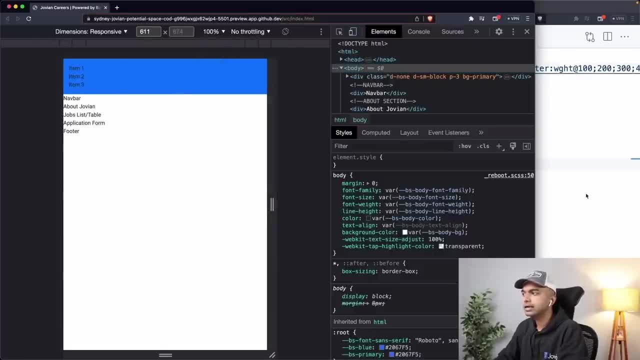 pixels. then this becomes visible And you can see that it is using the layout block, SM block. And let us add DMD flex here so that when we cross 768 pixels it should show up as a flex container. So all its items should go into a row and you can see now that it's items have gone. 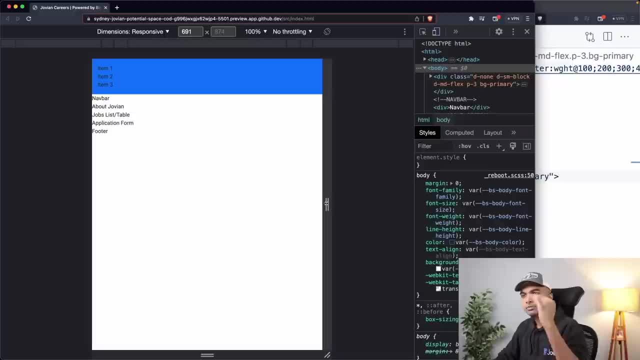 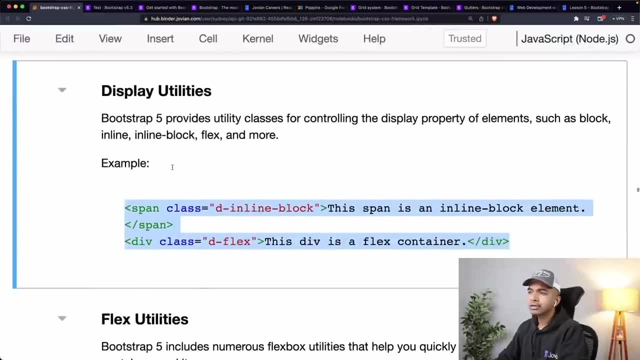 into a row. Okay, If I come back at SM, it is blocked. So it's item show one below the other and it is just not visible on a small screen, on excess screens. Okay, So these are the display utilities, very useful for just hiding and displaying things. 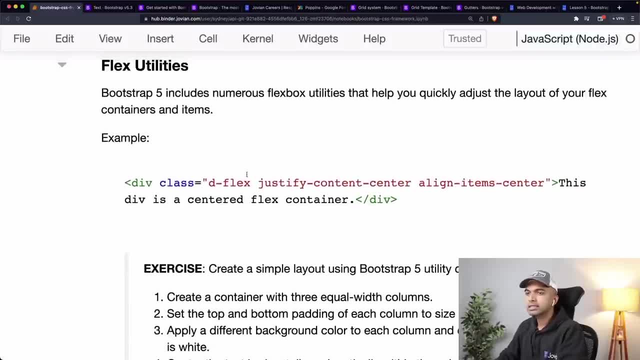 Sometimes you may want to do it the other way around, Yeah, So it also contains a bunch of utilities around flex box, So one of course is D flex or DMD flex or DSM flex. So all of these utilities, you can trigger them at specific breakpoints. 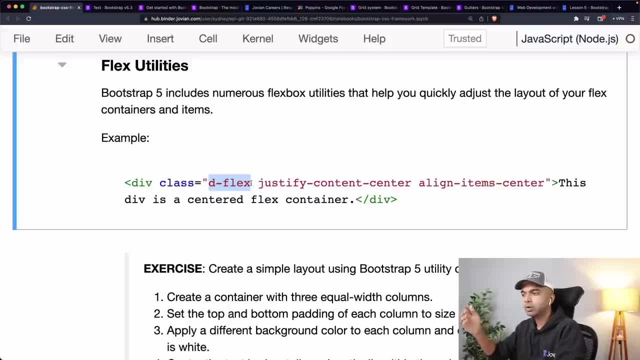 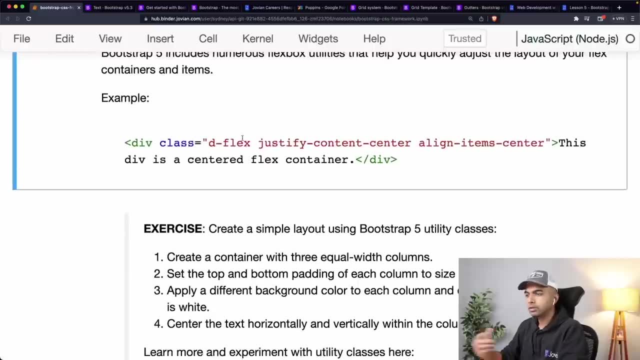 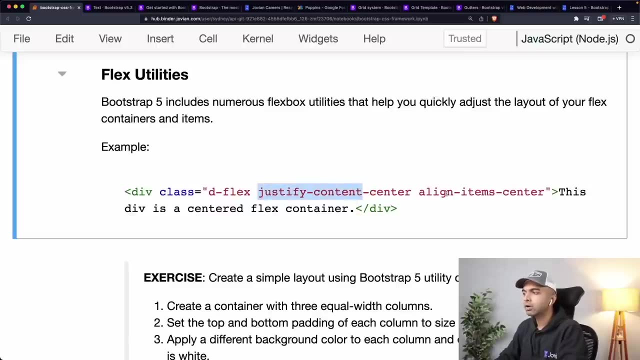 So you can say D, hyphen MD or BG, hyphen MD, hyphen blue or primary, et cetera, And all of these utilities can then also- and there are a bunch of flex box related utilities as well- Specifically the few, the two you might use and are justify content and align items. 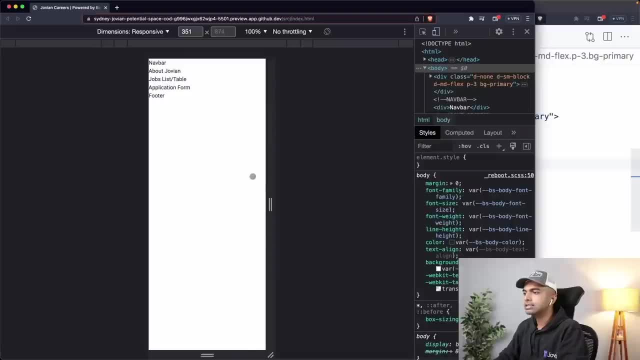 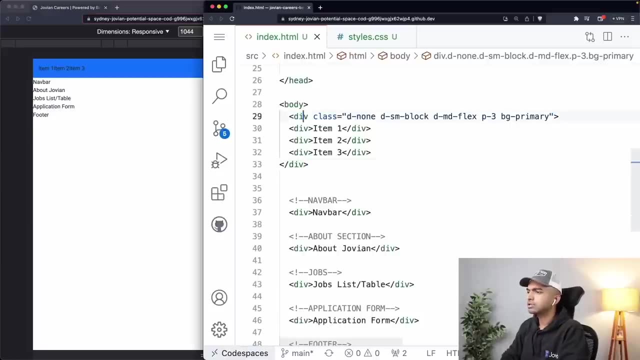 Okay, So let's just take a look at an example of this. but here these are now. this is now a flex div. Okay, And let me just also give it a big font size. Yeah, So this is now a flex container at MD screens. 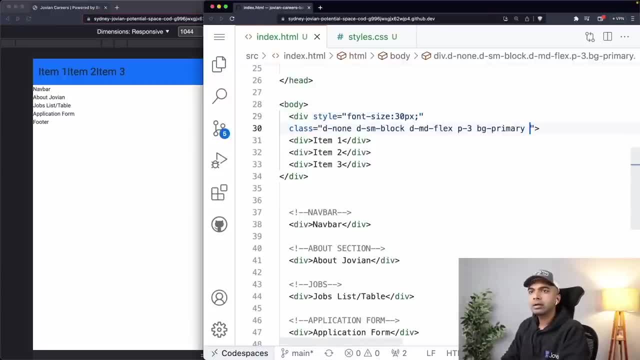 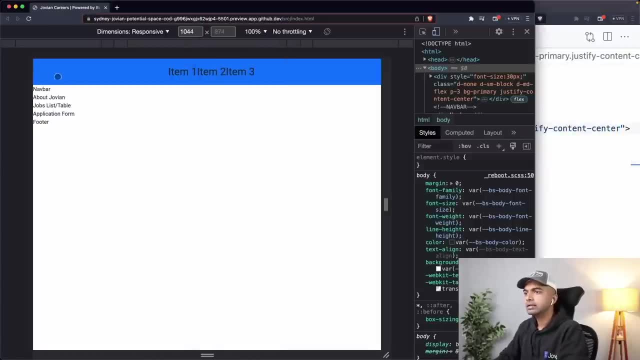 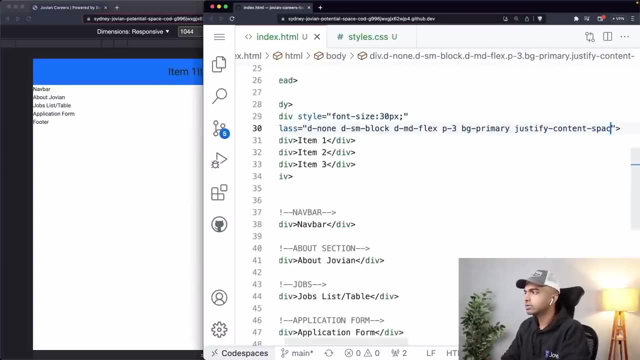 And I could do something like this. I could say: justify content: Okay, Okay, Center. And now you can see that along the main axis, because flex direction is row, by default, all the content is justified at the center. or I could say space between, or I believe it's. 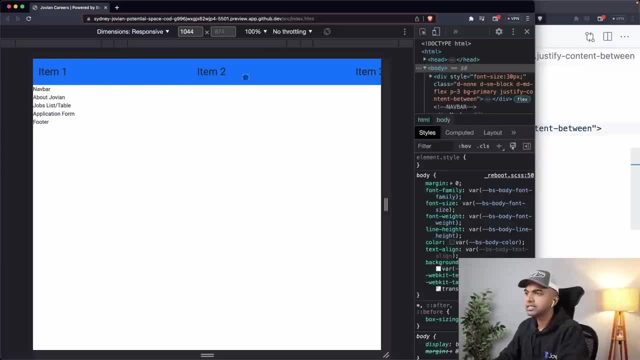 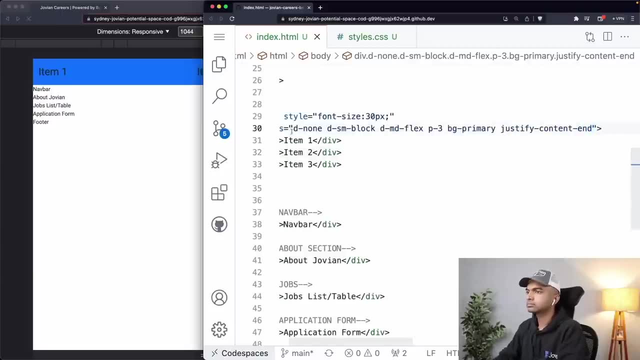 just between Yeah, So now we have added space between the content. So that is the other way this can work. or I could say: justify content, end, And now all of the content is justified at the end. Similarly, you can have a line items. 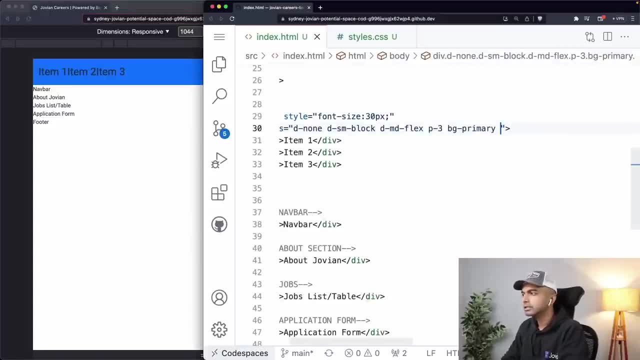 Okay, So let's say we give this a height. So let's say we give this a height of 300 pixels. Now I could do this. I could say: align items, end, and you can see that items one, two, three have all moved. 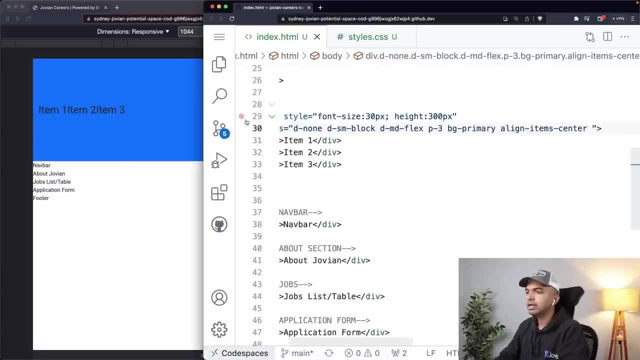 to the end Right, And the most common use case would be probably a line item center, where you want to center them along the cross axis, And sometimes you want to combine that with justify content, Enter, And what that essentially ends up doing is it. 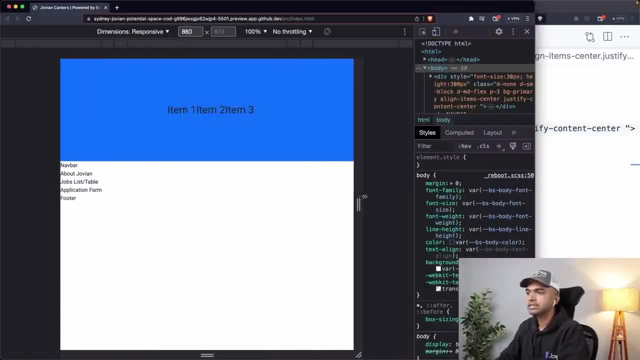 It centers no matter where you are And of course the flex gets triggered only at at LG or at MD. but no matter how you increase the height or width of the page, the content is going to remain centered vertically and horizontally. Okay. 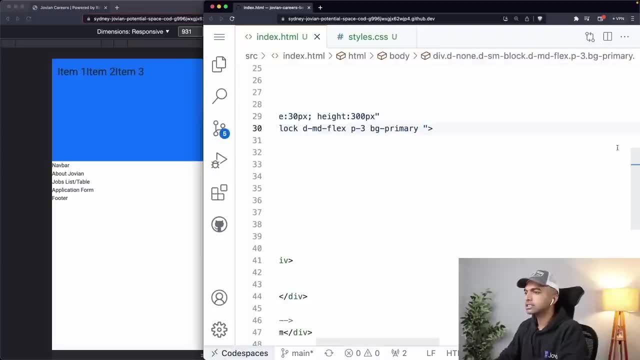 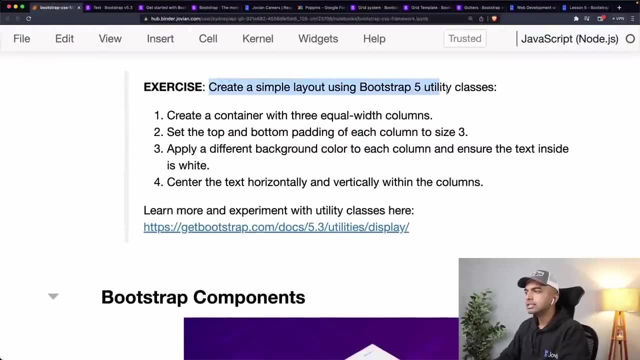 So you have all these nice utilities where you don't have to go into your styles dot CSS at all. You can simply just add them at the class level in the HTML. So I encourage you to create a simple layout using the bootstrap: five utility classes where 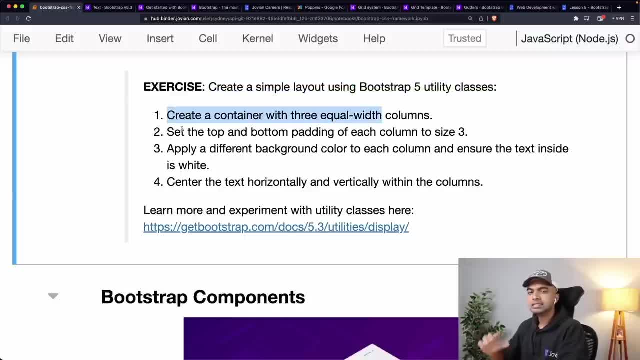 you create a container with three equal width columns, then set the top and bottom padding of each column to size three and then apply a different background color to each column and ensure that the text inside is white, And then try to center the text horizontally and vertically within the column. 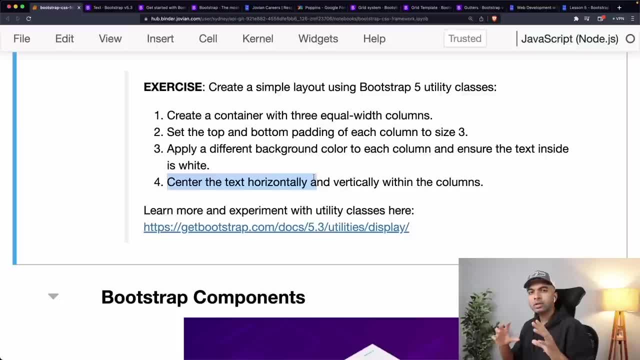 So try to do all of this and make sure, and also maybe throw in some changes at specific breakpoints and make sure that you are able to do all of this without writing anything within the CSS file. Okay, Okay, And you have to achieve a certain layout just using bootstrap CSS utility classes. 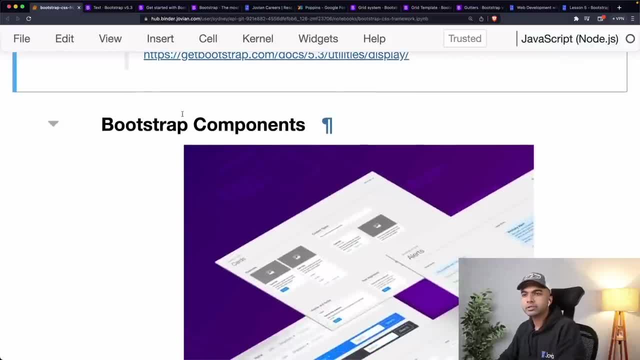 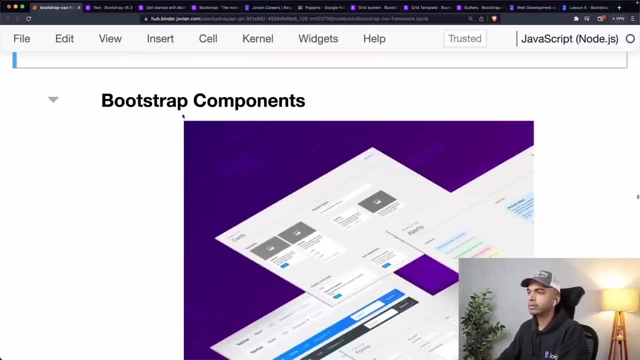 And let's see if you can do that. The way to become comfortable is just to exercise. There's no way you can remember all of these things. It's just the more you use them, the more they get committed to memory. We've now learned about the bootstrap grid system. 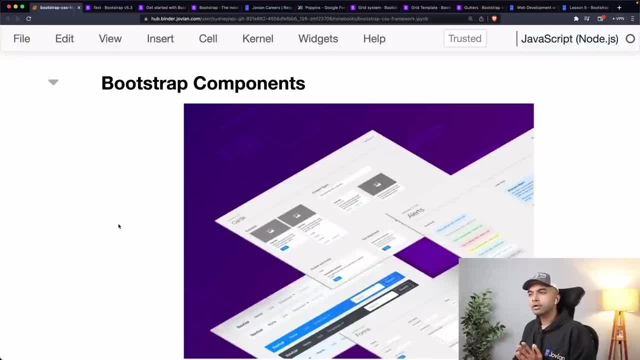 It's pretty extensive. It allows you to do a lot of interesting things. We have learned about bootstrap utility classes. They allow you to apply textiles, background styles, flex styles, distribution styles, etc. Now we are in a position to actually start building out our page. 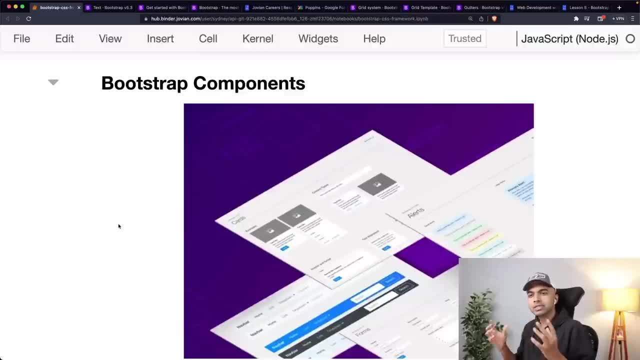 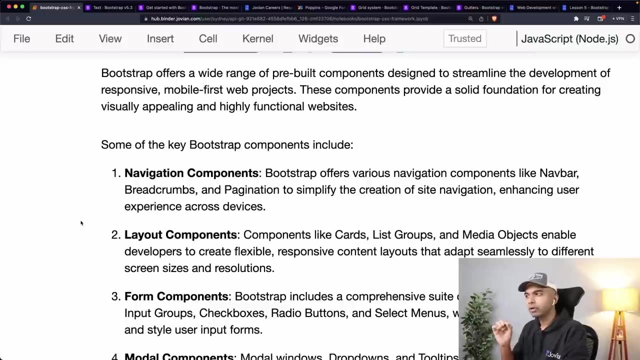 And we're not going to write the HTML of our page from scratch completely, in the sense that we're not going to just use grid and styles. we're actually going to use some components that the creators of bootstrap have already put together for us. Okay, so bootstrap offers a wide range of pre built components. 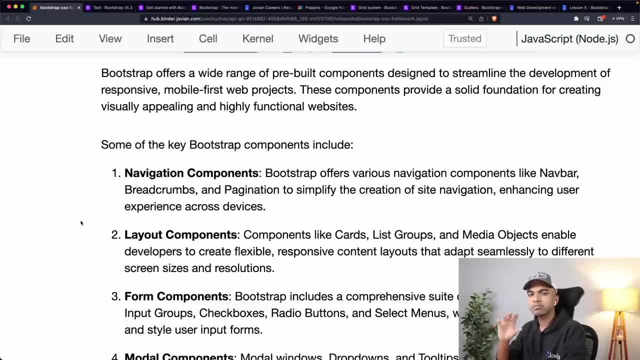 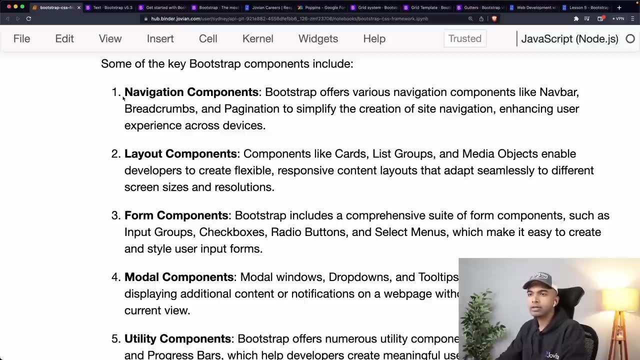 And these components are designed to streamline the development of responsive mobile first projects, And these components provide a solid foundation for creating visually appealing and also highly functional websites. Now, there are a bunch of different components and we'll go through various. we'll go through some of them, definitely not all. it's a huge library with a whole bunch of components. 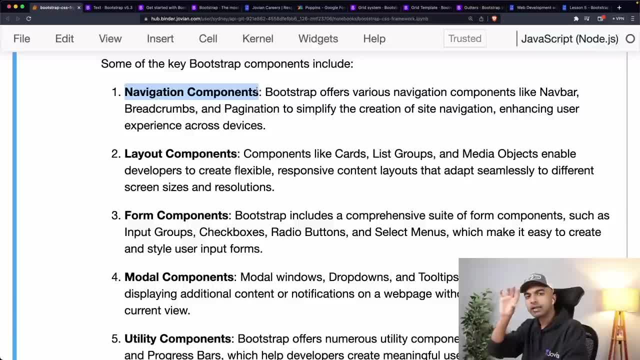 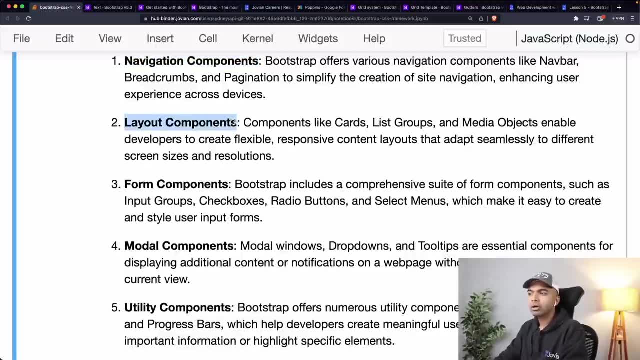 But the few categories are navigation components, So things like navigation bars, headers, footers, breadcrumbs, pagination. that is something that we'll find in bootstrap. then there are layout components, So you can create cards, you can create list groups. 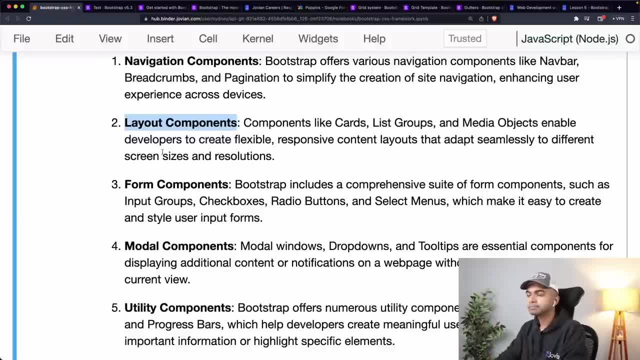 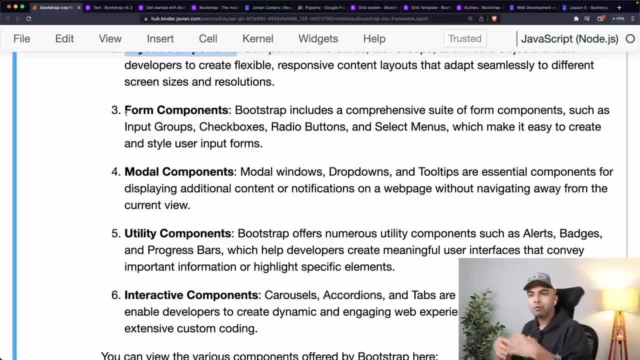 You can create media objects like images etc. There are a bunch of form related components, So the creators of bootstrap have set up some special classes for rendering forms nicely, so that you don't have to do a lot of work to show forms on your web pages. 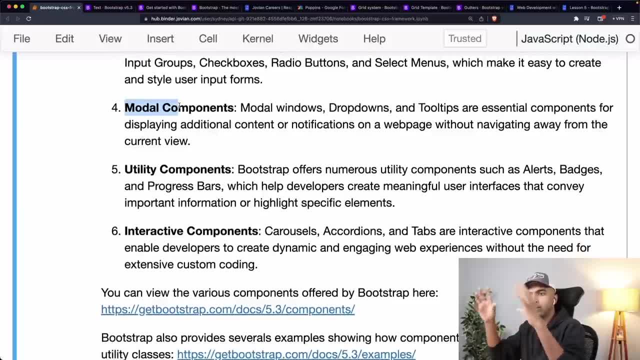 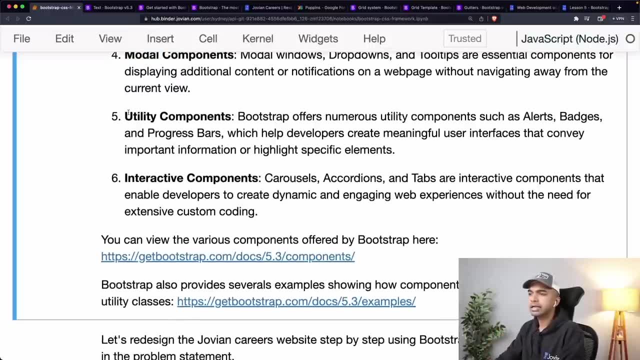 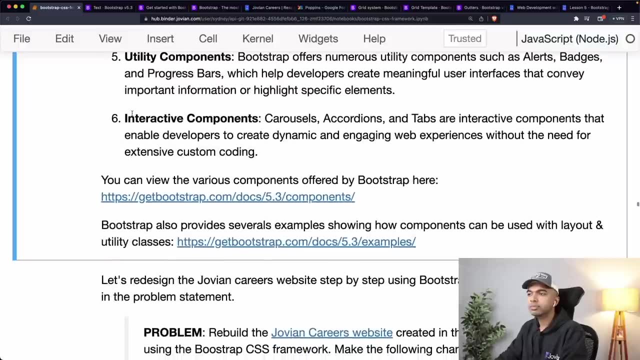 There are a bunch of modal components, which is basically pop ups that overlay the entire screen or things like drop downs and tooltips that you can add. Then there are, of course, like a bunch of utility components like small alerts and badges and small things that you can use to highlight important information within your page. 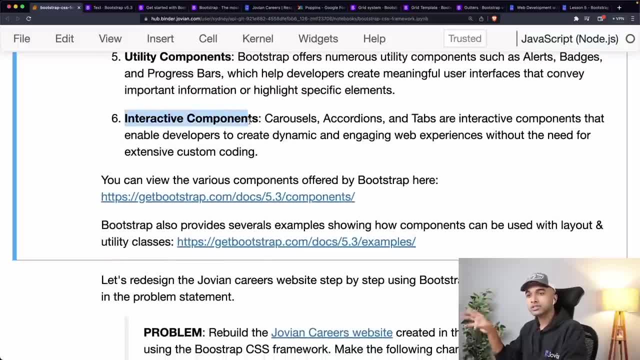 And there are also a lot of interactive components, And this is where a lot of the JavaScript is used, Because, remember, we used, we imported a JavaScript module as well. So that's where we have, like, accordions, carousels tabs, etc. 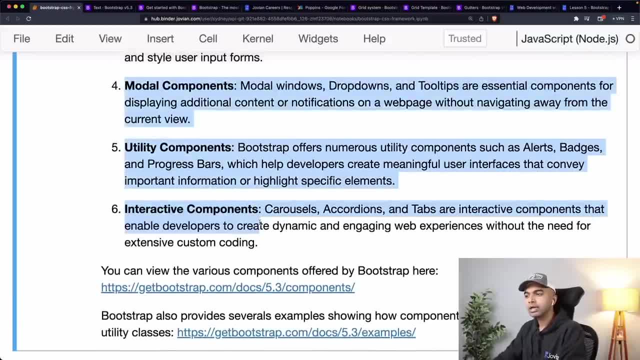 And I encourage you to check out these three. we're not going to cover them today, So they will possibly be get covered as part of a future assignment or something, But I encourage you to maybe play around with these a little bit, Okay. 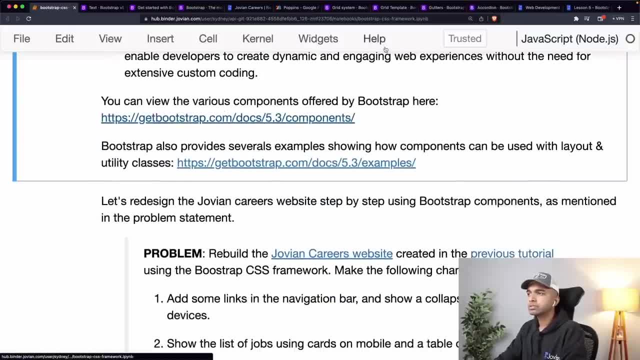 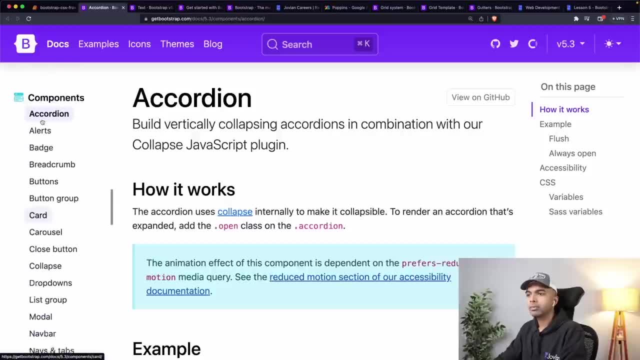 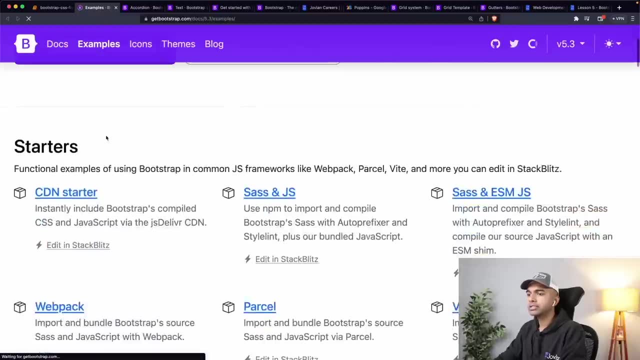 So you can check out the various components offered by bootstrap here. So bootstrap has this section called components in its documentation And there are a whole bunch of components that you can pick up, So I'll let you check these out. And then there are also several examples on bootstraps web page on how to use these components. 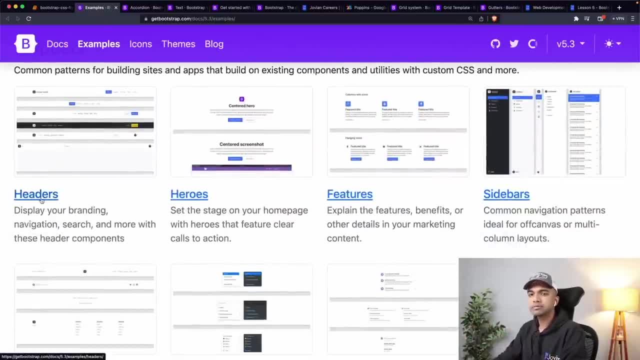 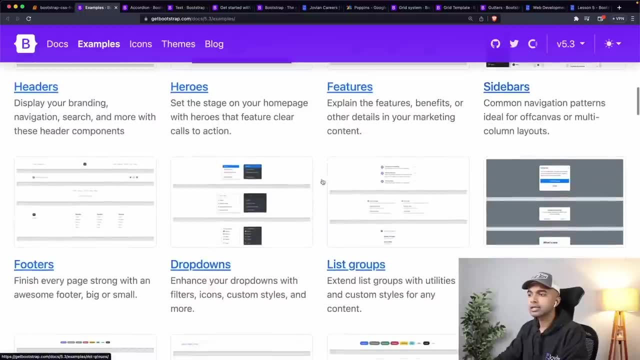 in a proper page. So here there are some common patterns for building headers, navbars, building the hero or sort of the main section, maybe building some feature sections, building sidebars, so you can create all sorts of interesting layouts using bootstrap components. 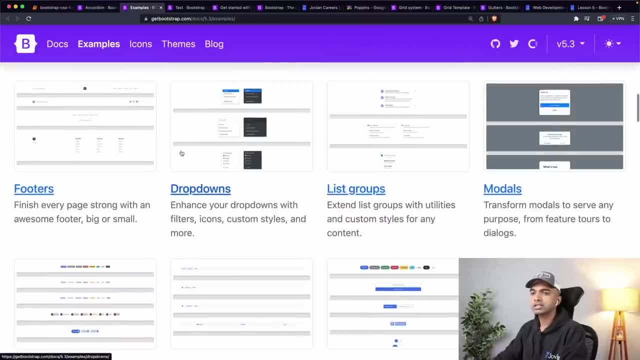 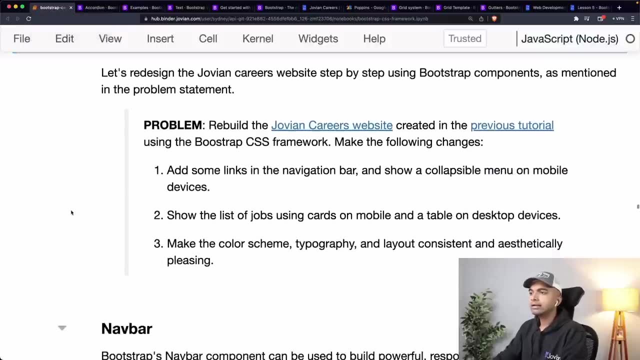 So check out the documentation for components and maybe also check out examples. So whenever you're working on a project, these two pages are going to contain a lot of useful information for you. So with that, let us redesign the Jovian careers website. 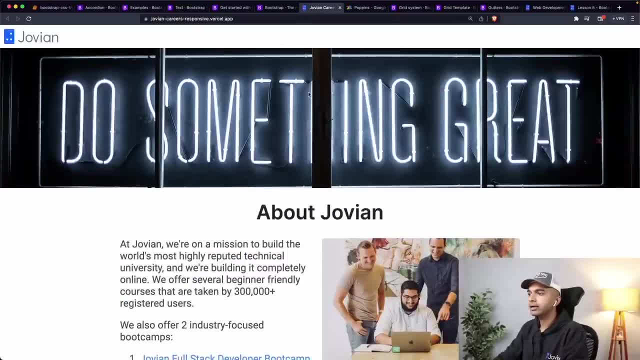 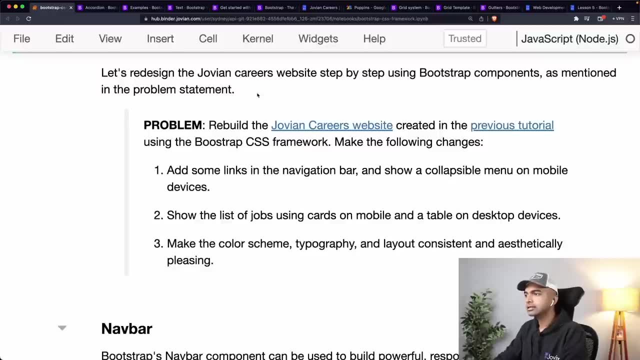 So this is the Jovian careers website right now. This is what it looks like: There's a navbar, there's a banner image, there's about section employment opportunities, submit your application, etc. So let's redesign the careers website step by step. 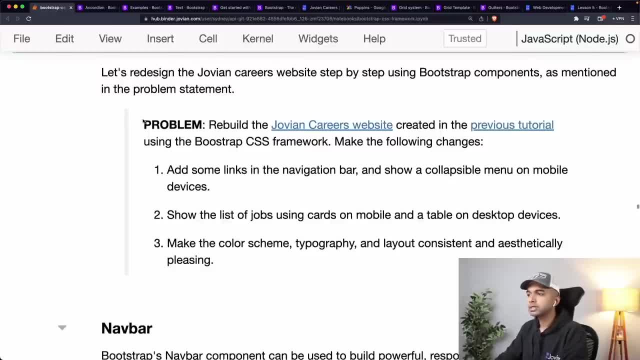 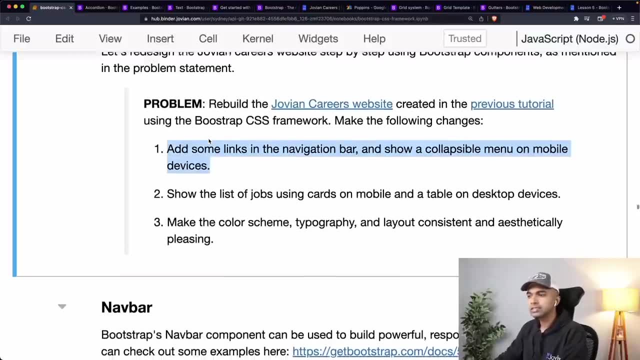 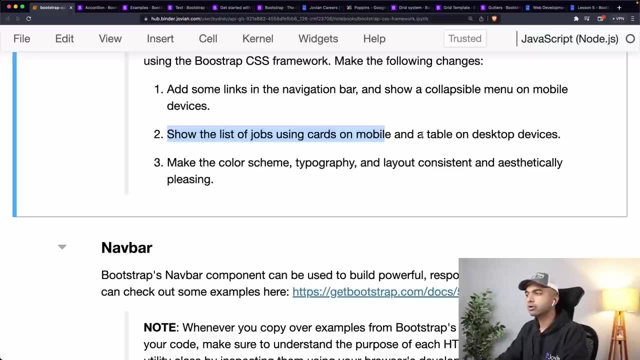 Using bootstrap components, as mentioned in the problem statement. So the first thing we're going to do is we're going to add some links in the navigation bar and show a collapsible menu on mobile devices. We'll see what that means. We'll also show a list of jobs using cards on mobile and on desktop we're going to use 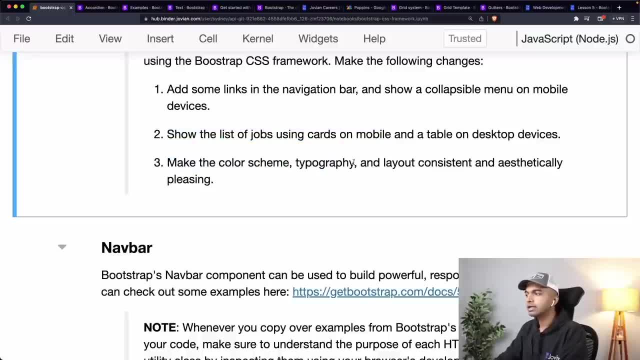 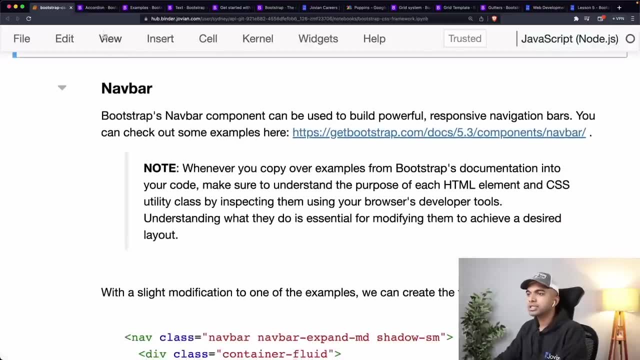 a table and we're going to make the color scheme, typography and layout consistent and aesthetically pleasing. Okay, so let's start with the navbar, And this is where we can use bootstrap's navbar component, So we can come in here and you can see here that there's a component called navbar. 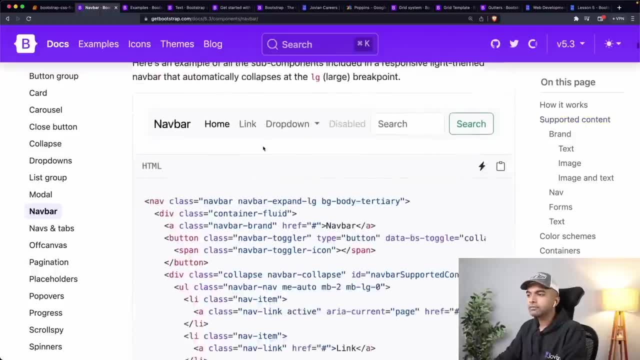 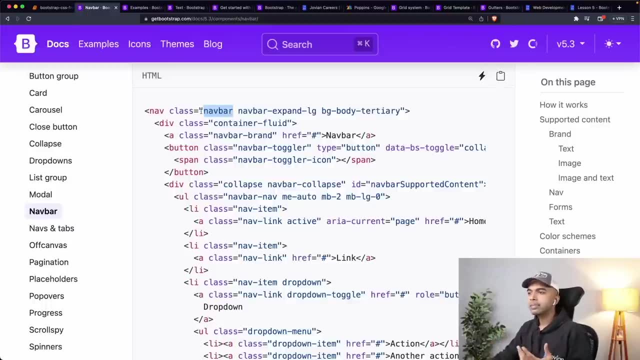 And a component essentially is simply a bunch of HTML and CSS along with some special classes. So the way you use a bootstrap navbar is basically by adding a class navbar to a nav element And there are a bunch of classes that need to be added. 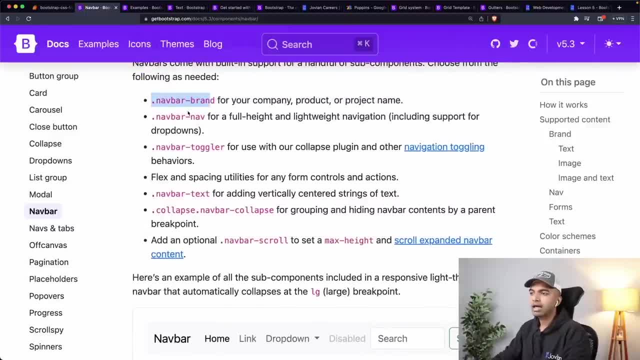 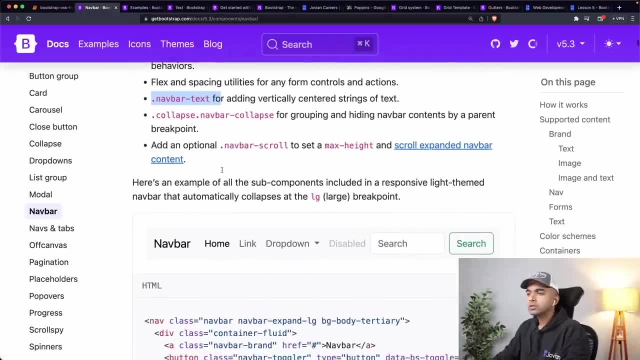 So the information about the classes that need to be added are here. There's this navbar brand, navbar nav, navbar toggler, navbar text collapse, etc. So we can come in here. Okay, Navbar scroll. So the best way to actually do this is to maybe go through the examples that have been. 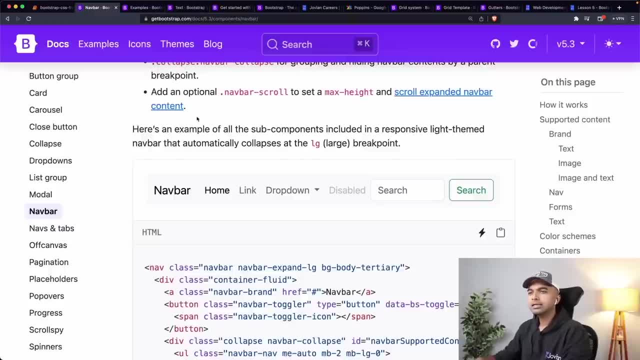 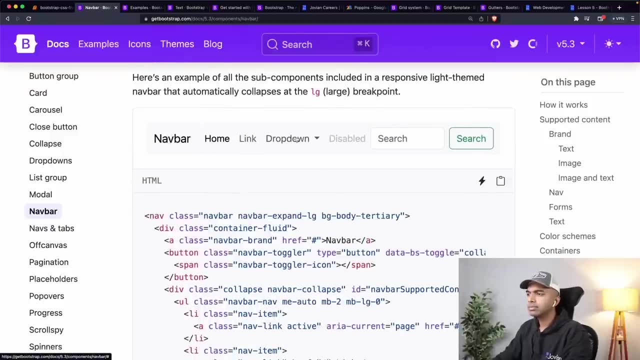 given on the page and pick the example that is closest to what you want to achieve. Okay, so here is a navbar which contains this. maybe this could become the logo and maybe these could become the links. We don't know this form as such. 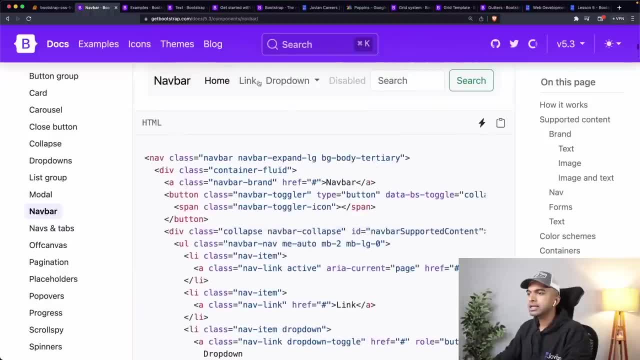 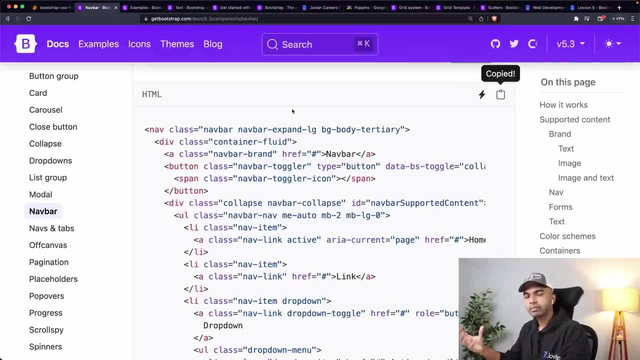 So we may not need this, But there's an. so this is an example, example: navbar- And this is the code for that example. So what you can do is you can simply copy this code And paste it. Now, remember, whenever you paste code, you should study it line by line to know exactly. 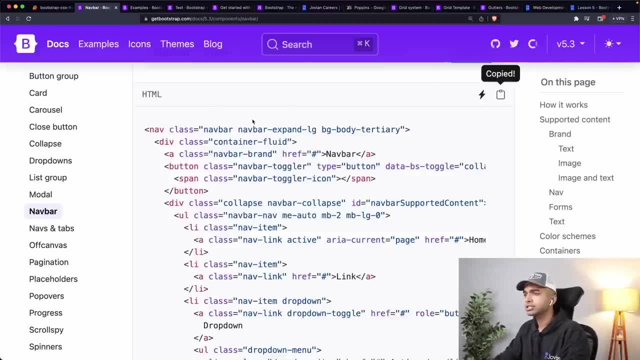 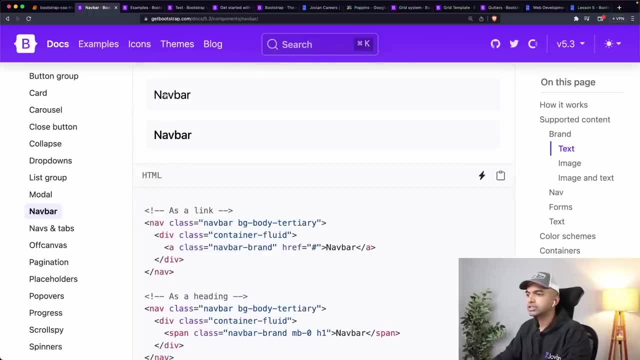 what it does. Okay, So copy this code and paste it in your HTML And that will give you a navbar. And there are also various other examples. So this is like a plain navbar, simple navbar. you can check out these two as well. 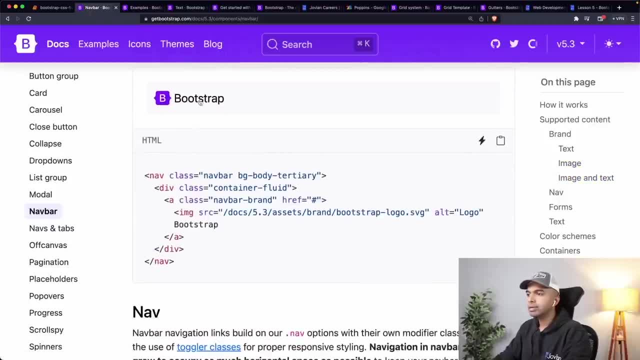 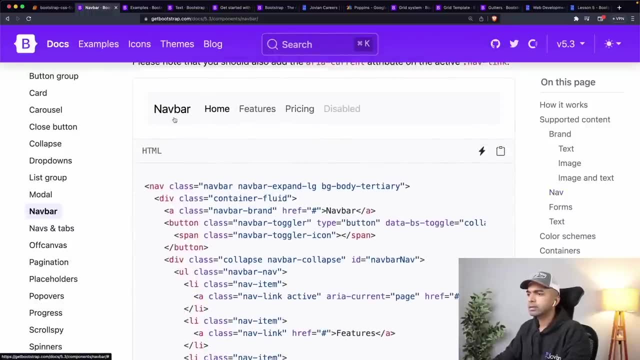 This is a navbar with an image. This is a navbar with an image and some text. This is a navbar with just a bunch of links. I think this is something that we might be able to use, And then there are a bunch of links. 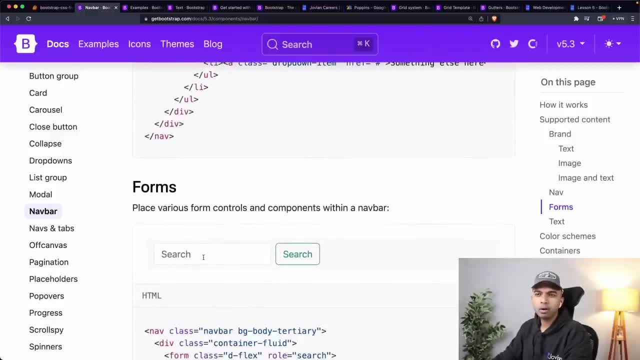 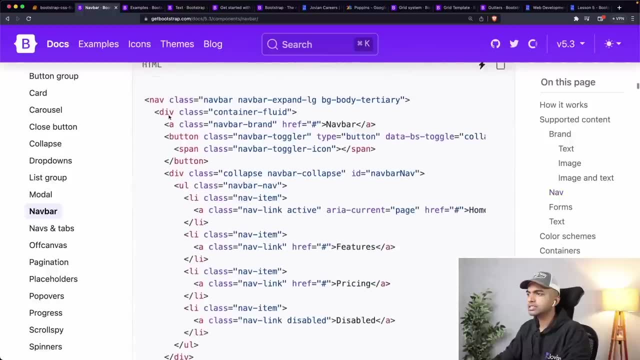 Okay, So there are a bunch of different examples. So you can. you can also embed forms within the navbar. I think I am simply going to maybe just pick the first. let's pick a very basic one navbar with a bunch of links, because that's what I want ultimately. 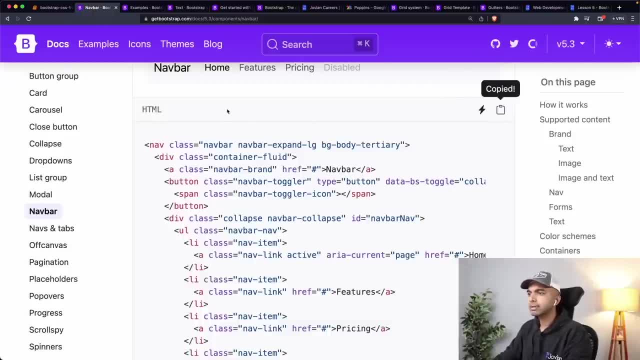 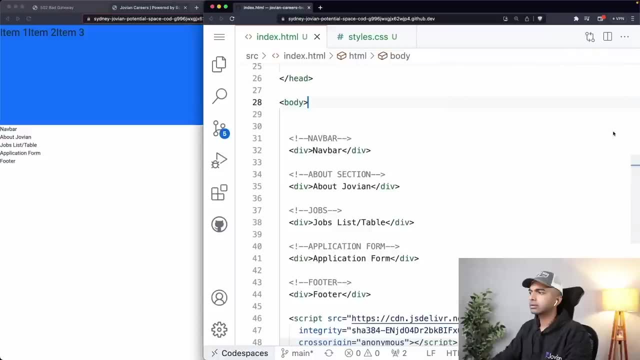 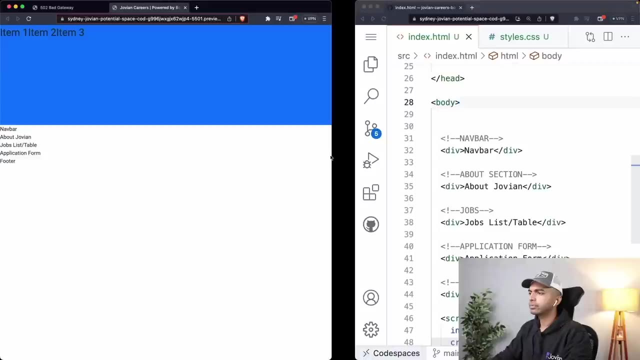 So let me pick this up And let me start customizing it step by step. Okay, Let's get rid of this And let us just maybe bring this: make this a little smaller And make this a little smaller as well. Let's reload this. 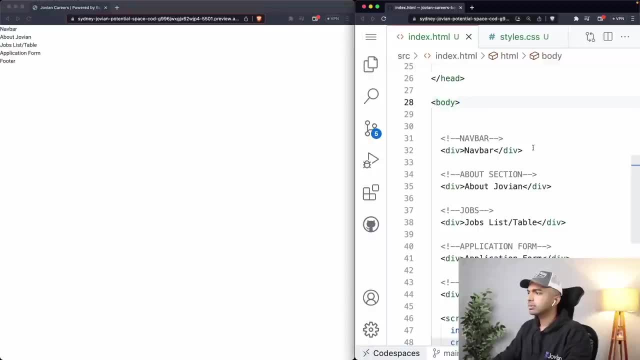 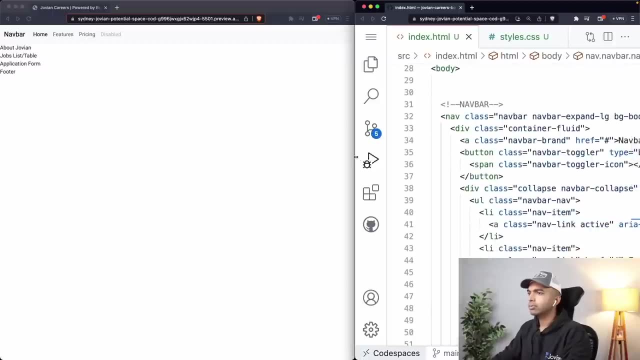 Okay, So this is what we have. No change here. Now let me just come in here and replace this navbar div with the code that I've just copied over. Okay, So this is the code that I've copied over, And this code results in this navbar being added to my page. 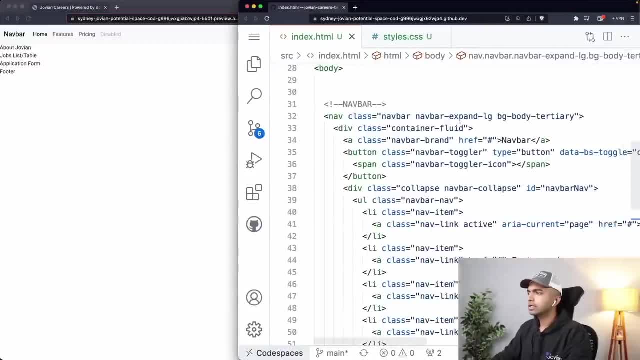 All right. Well, so first thing I want to do is I'm just going to study it line by line and I'm going to make some changes to it. So, all right, I have this class navbar and I want this navbar to show. 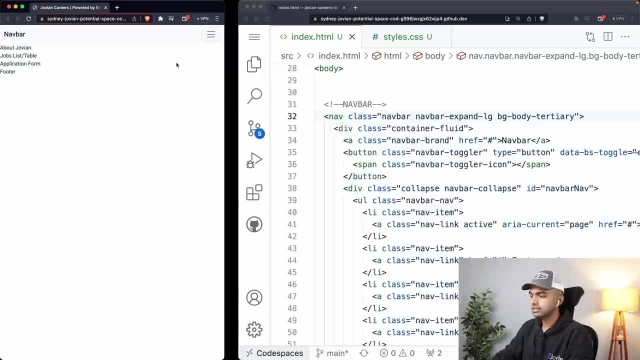 So it's going to show up in a collapsed form like this. You can see that there's a button here, There's a button here And when I click on this button it opens up this menu. So bootstrap automatically gives me this nice mobile dropdown menu so that on mobile there's 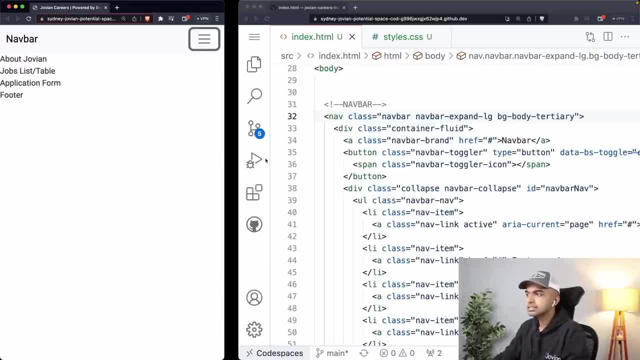 no space to show the links, So it's going to show up in this button. So that's nice. Now I want to specify when I want it to expand. do I want it to expand on small screens, medium screens or large screens? 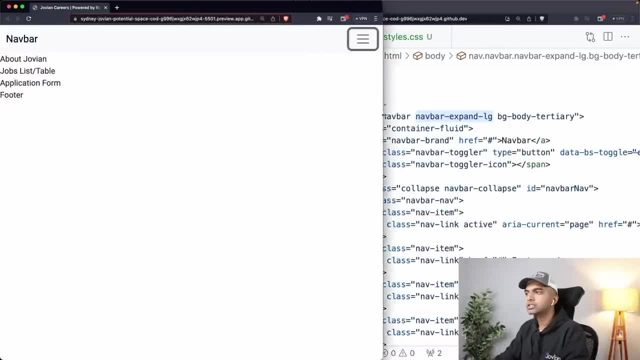 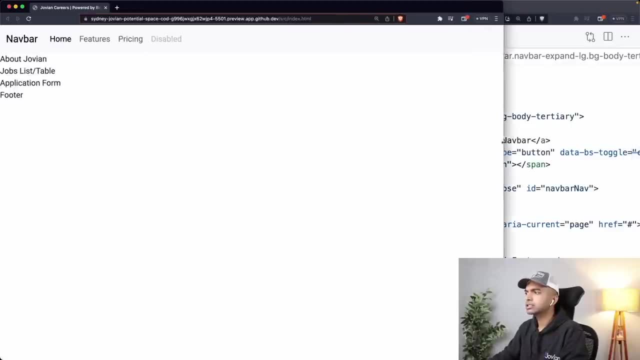 So currently it is set to LG, which means when the width of the page crosses nine- 92 pixels, I'll have to maybe zoom out a little bit, Yeah, But when the width of the page crosses nine, 90 pixels or so, then this gets shown normally. 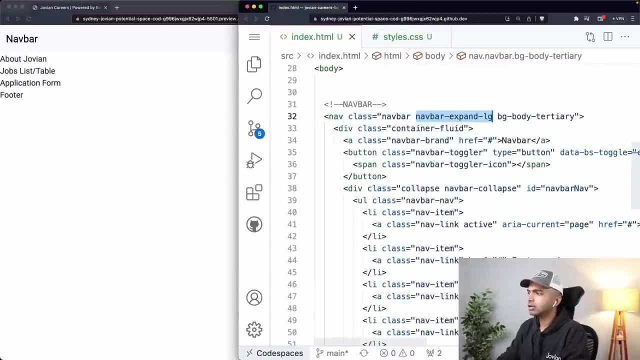 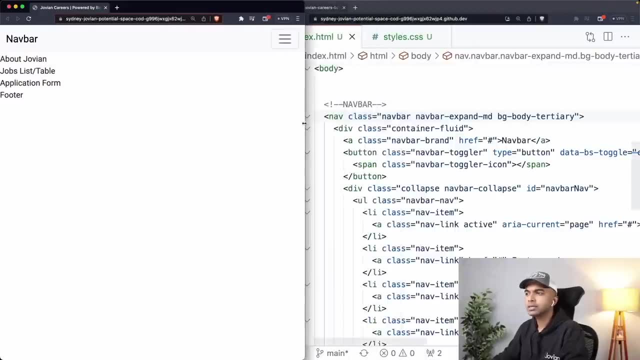 Otherwise this gets shown like this: Maybe I don't need to expand LG, Maybe I can do with expand MD. So yeah, So you can see here that up to the MD Breakpoint, which is about seven, 68 pixels, It's going to show up like this, and after the MD breakpoint it's going to show up like: 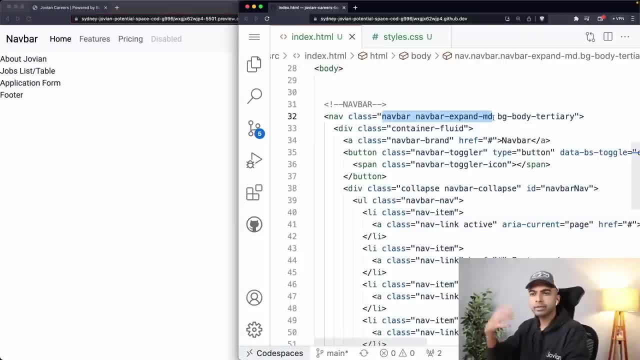 this. Okay, So that's what these two classes mean. Now, bar is simply going to trigger the entire navbar component for this particular element And then the BG body, tertiary, I believe this is simply the background color. I don't need that. 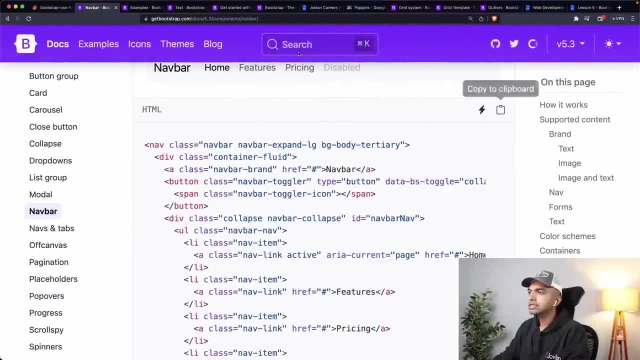 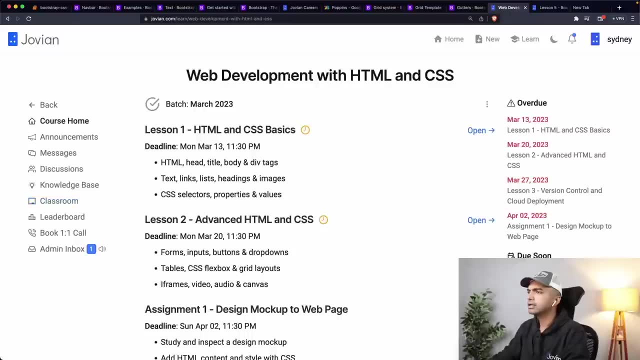 So I have gotten rid of the background color. What I do want is I want to add this nice shadow. I want to add like a small shadow here, which I have, which we have- Okay, We have on the Jovian website. you can see that we have this nice subtle shadow below. 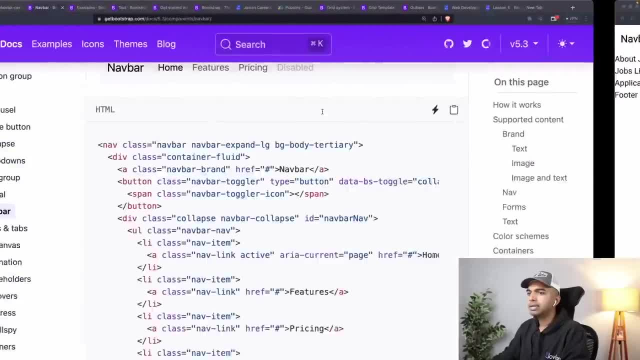 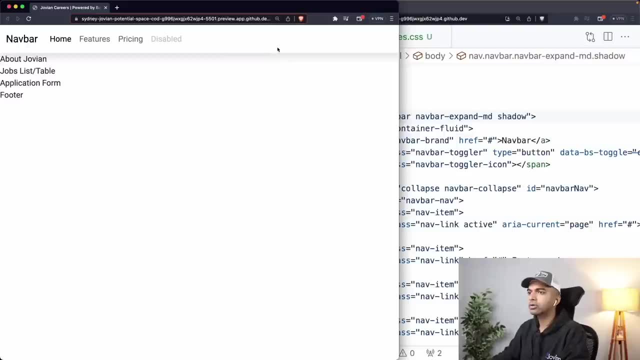 the navbar. So I'm going to try and add that shadow And I believe there is a utility class for adding shadows. I believe you just say shadow and that's going to add a utility shadow here, but this shadow is too big. 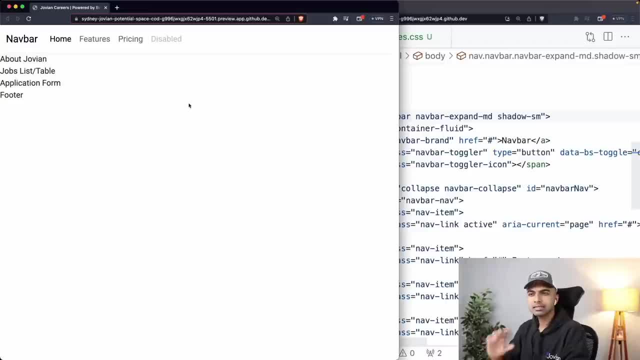 I can make that smaller. So there's like a shadow SM utility class again, something that you can just search online how to add a shadow and bootstrap, and you can just find it online on Google or chat GPT. Okay, So now. 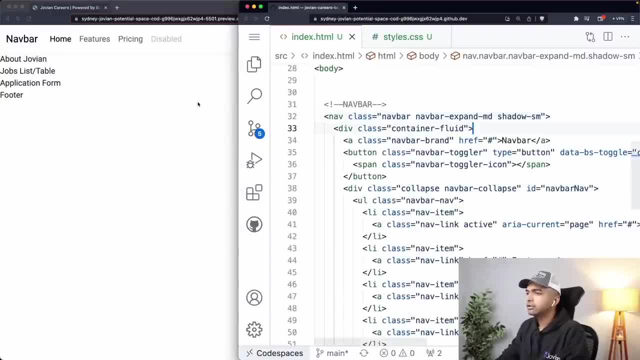 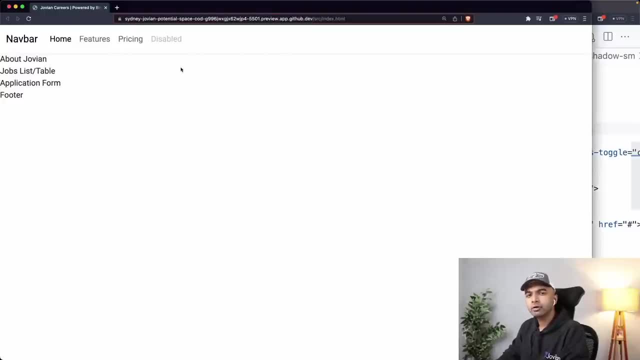 Okay, That is nice. Next, we have this container fluid, So we have this navbar. it's going to take up the full width of the page. What do I want? Do I want it to take the full width of the page? 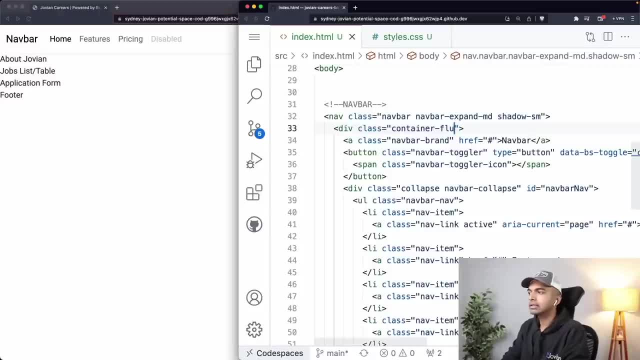 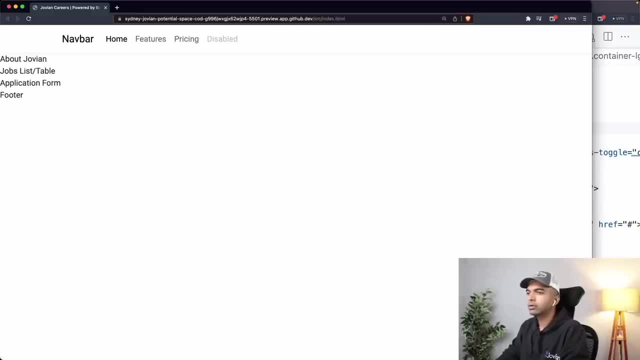 Well, maybe I wanted to take the full width of the page till the medium screen, But for LG and bigger, I want it to be centered. Okay, So I'm just going to do this. I am going to pick. Yeah, so I'm just going to maybe make it fluid. 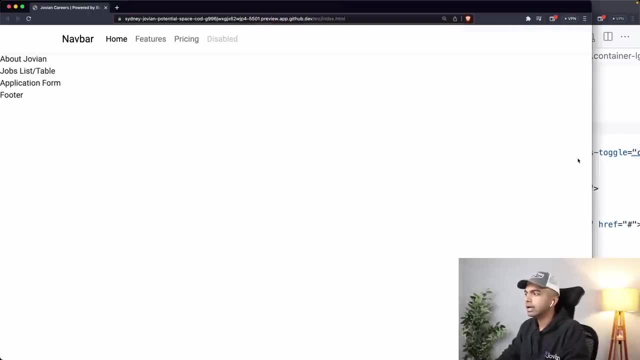 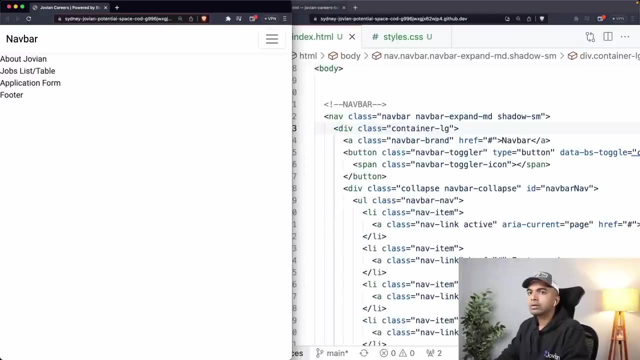 I'm just going to make it center, Okay. So I'm just going to make it LG at LG, it's going to become centered And it's going to remain fluid for MDN below, okay, So remember what this container is doing is. this container is deciding whether the 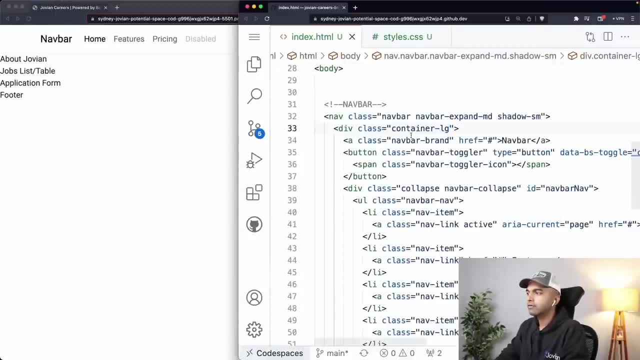 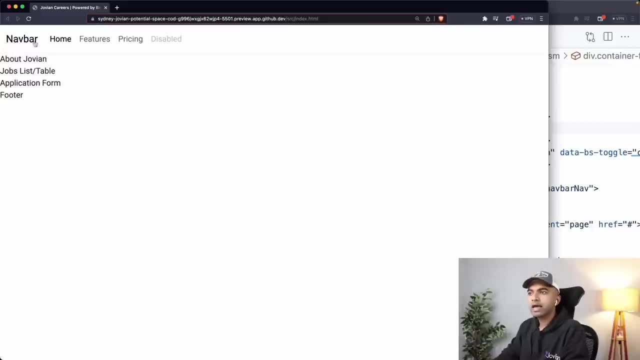 entire navbar should be centered on the page or not? Now, if I don't have this container LG, you will. or if I just make it container fluid, it's always going to span from the left edge to the right edge, okay, and that is different. 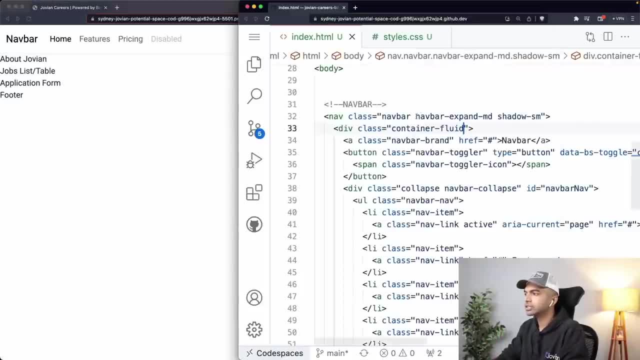 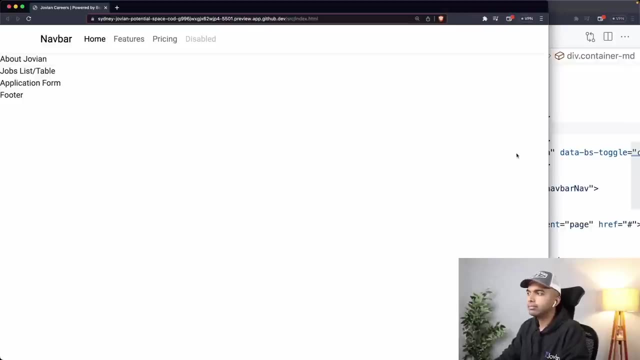 from the toggle: the toggle. The toggle is controlled using the. Okay, So now, if I expand the container, fluid decides whether the navbar takes the full width of the page or not. Let me just set it for now as container. I'm MD or container. Yeah, container MD. 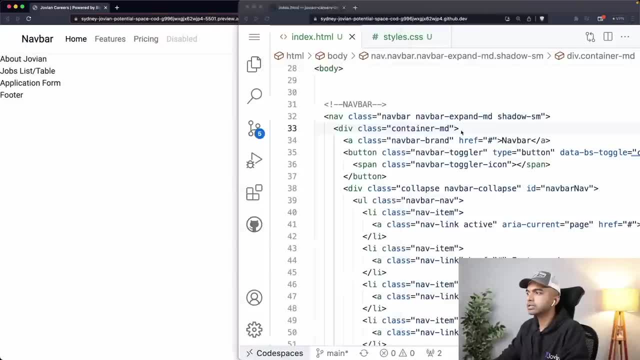 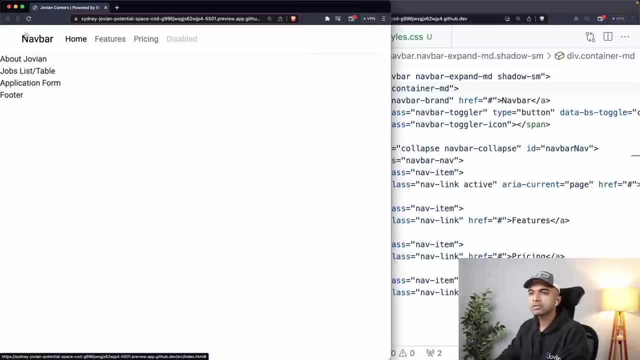 So from for MD screens and bigger, it is going to be centered on the beach, Okay, So that is what this does so far. This is fine. Okay. then we have this brand navbar. Okay, I think this is where I might want to put. 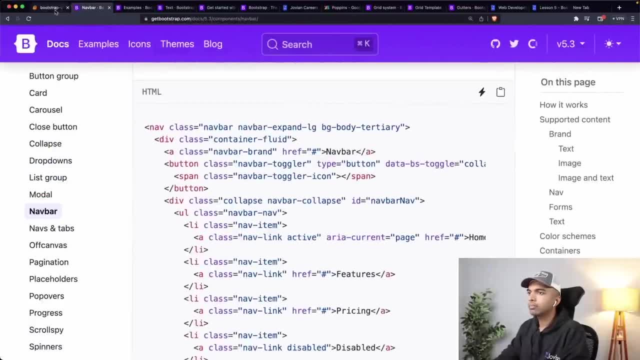 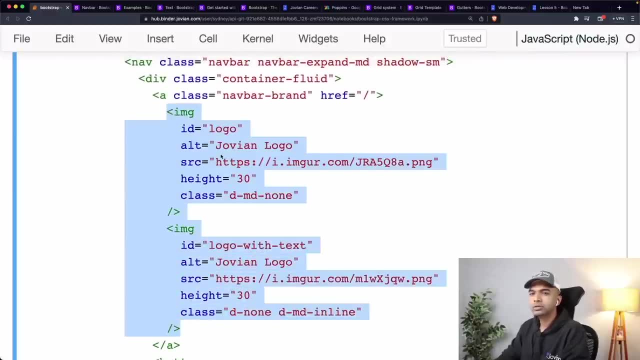 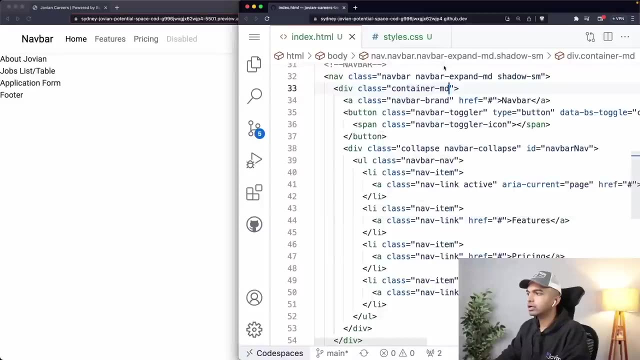 the Jovian logo. So I'm just going to grab the Jovian logo. So we have a couple of logos. there's one logo that is going to show up on small screens, which contains just the icon. does not contain anything else. 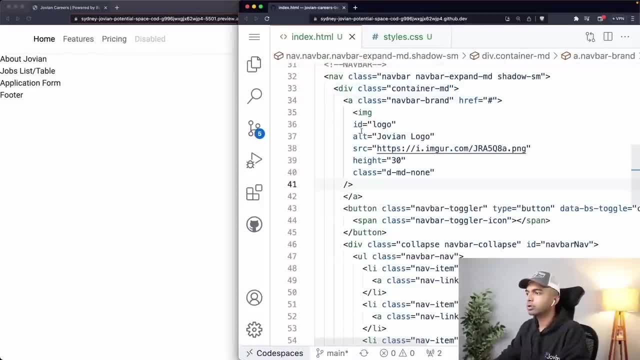 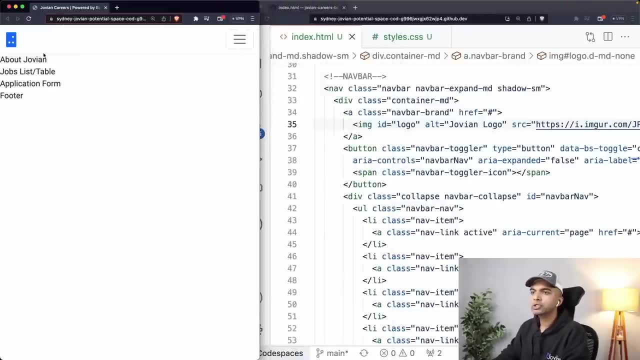 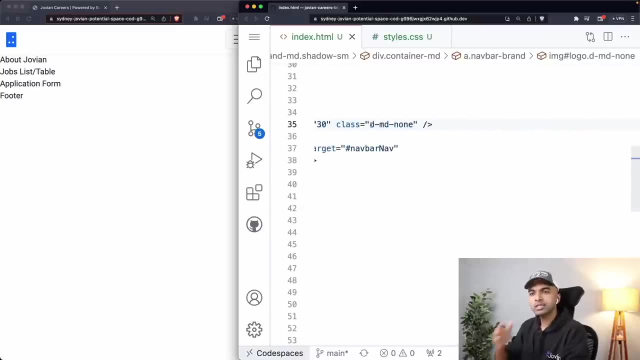 So let me remove this text navbar over here And let me just put the Jovian icon and you can see that it's going to show up on small screens, But as soon as I hit Yeah, So you can see that I have given it the class DMD none, which means it's going to show up. 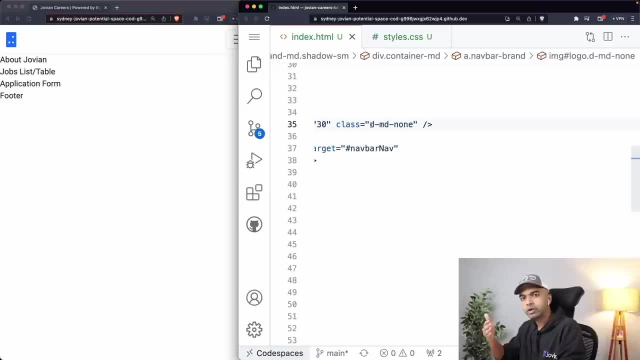 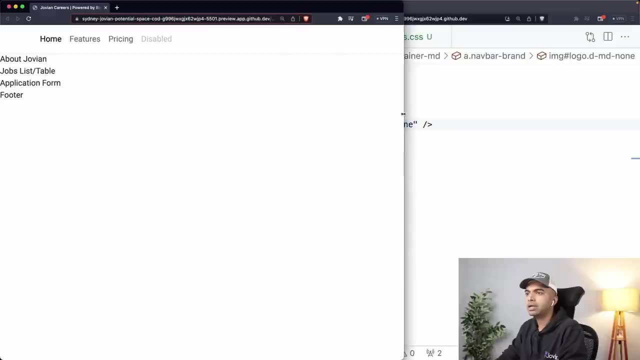 on small screens, But as soon as we hit the MD breakpoint it is going to stop showing up. Okay, And why do we have that? because for bigger screens or for MD breakpoint, actually want to show the full Jovian icon or the full Jovian logo with the text. 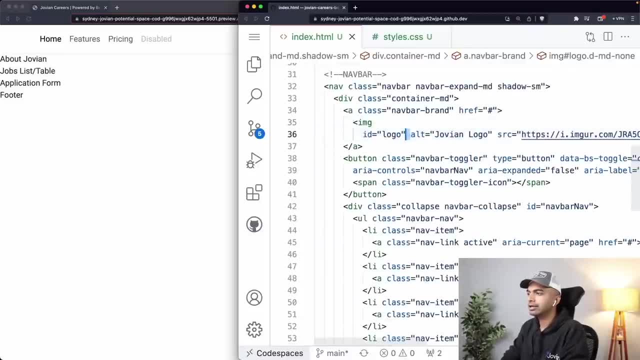 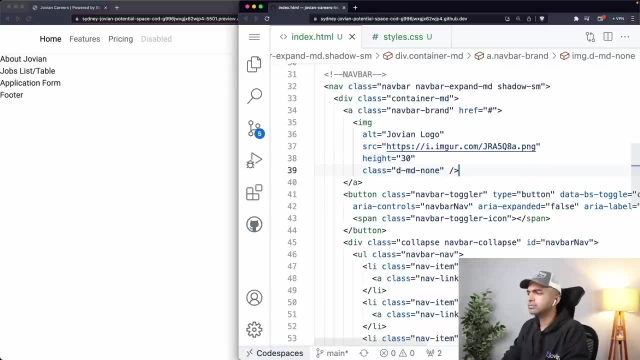 So let's put this in your. Okay, we're given it. I don't think it needs an ID anymore. So I think the ID can be gotten rid of, And even the height may not be necessary, but it's fine, Let me just keep the height for now. 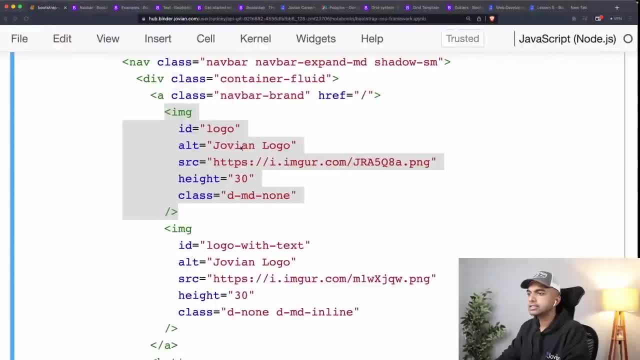 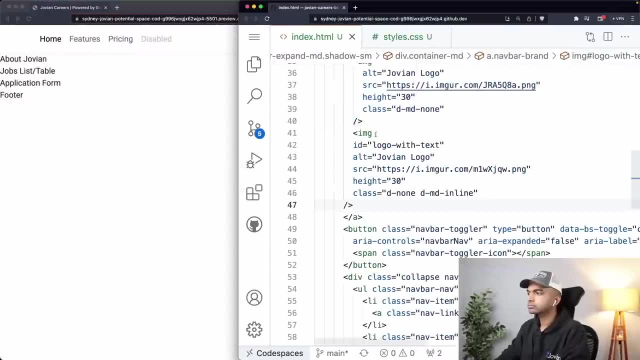 Okay, so let's get another Jovian logo for bigger screens. So let me grab the Jovian logo with text. So this is simply, again, the Jovian logo with text. So again, it's an image tag, And what we're seeing here is that it is hidden by default. 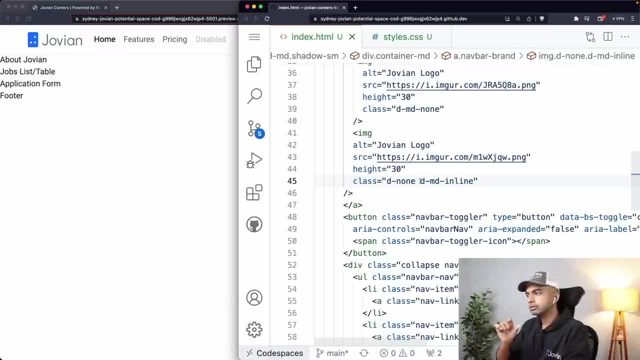 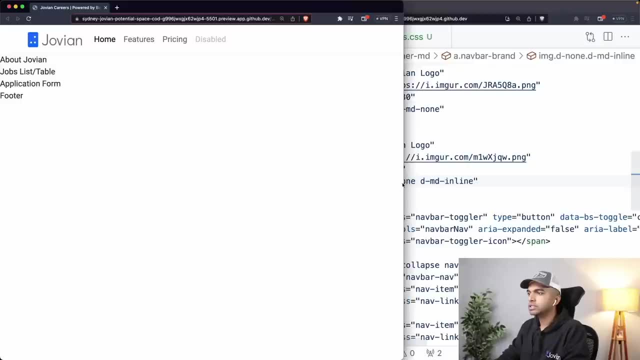 So it has a display of none, But from the MD breakpoint, which is 768 pixels, we wanted to show up in line. Okay, So this is what that ultimately results in: that, up to MD, we have the smaller logo which. 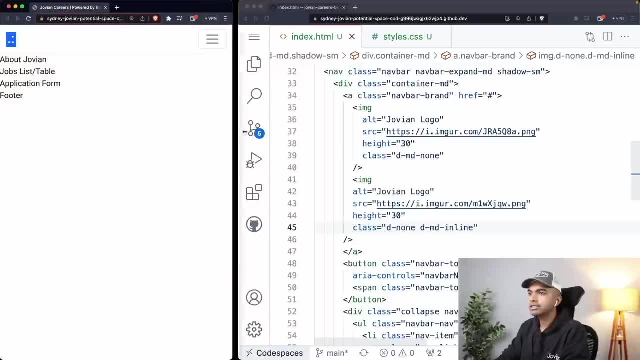 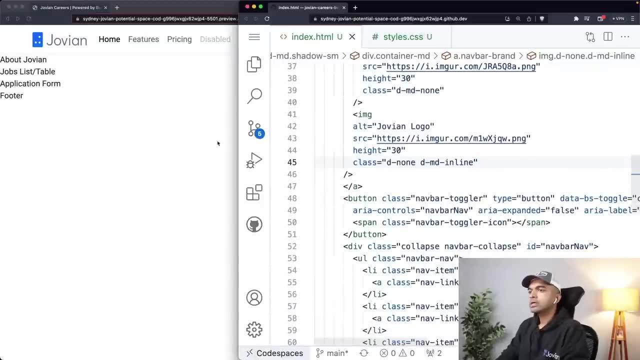 contains just the icon, And then, beyond MD screens, we have this bigger logo which contains the actual Jovian logo. Okay, cool. So our Navbar is almost ready. I think we're almost ready to go ahead. Let's see what we have here. 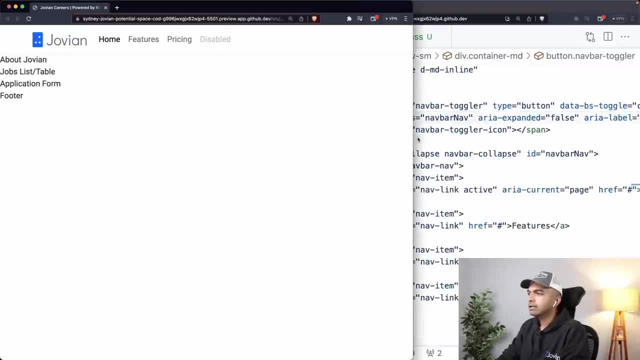 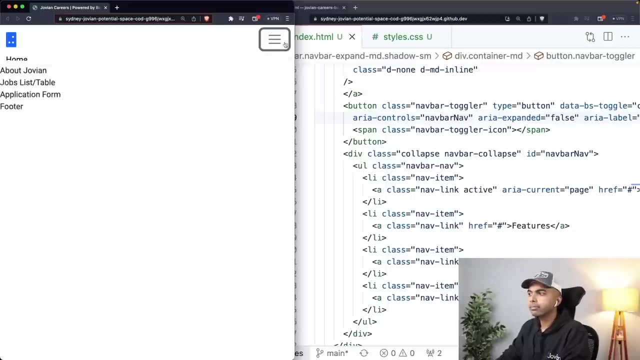 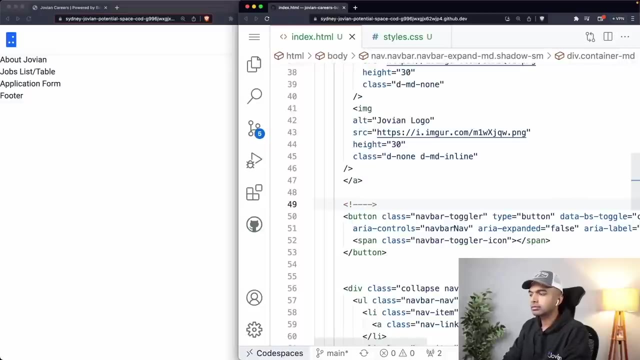 We have this Navbar toggler of the type button. If I understand correctly- I think it- what it's doing is basically simply Setting this button. So this button is the button that is rendered here. So this is simply the toggle button. but I can also maybe just add a quick comment here. 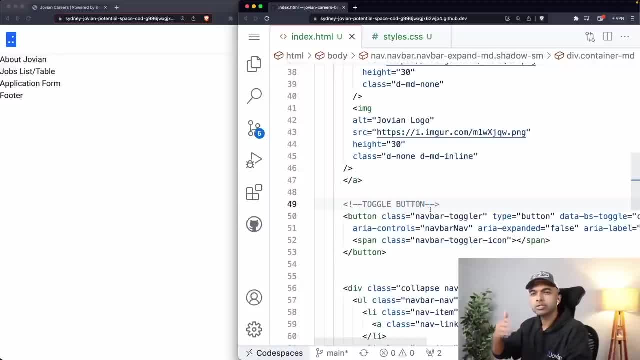 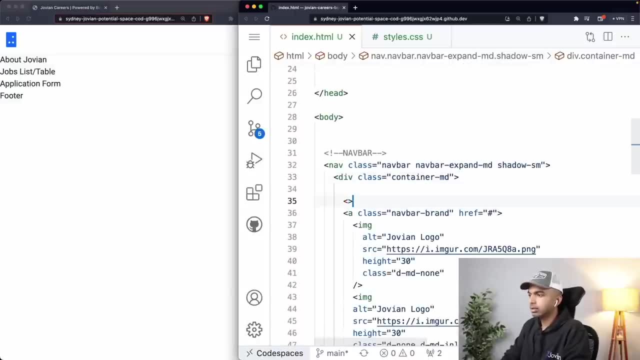 So this is the toggle button, And this toggle button only shows up till MD, because after MD it is going to just expand automatically. And maybe I can add a small comment here saying this is the logo. Okay, So now in my Navbar. 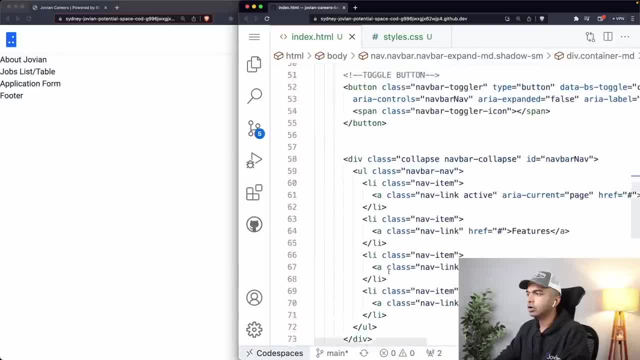 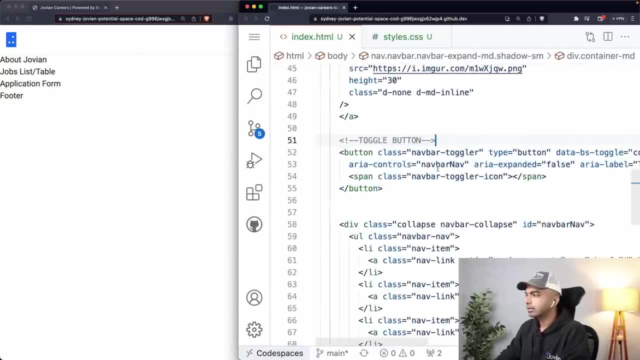 Okay, I have the logo and I have the toggle button. All of this is fine. Now, in the Navbar we have and in the toggle button we have this that it controls or it targets this Navbar nav, and the Navbar nav happens to be this div which contains: 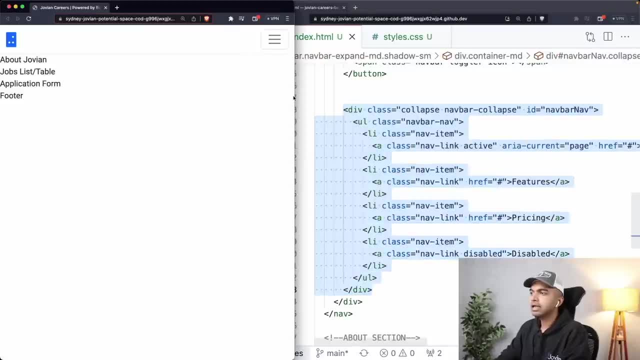 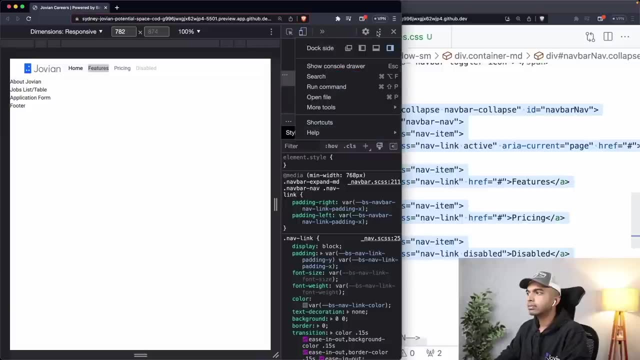 a list inside it. Okay, So it's not visible until we hit the MD breakpoint, And then, from the MD breakpoint, it becomes visible And we can verify this by clicking inspect. And let me just turn off the device mode for now. 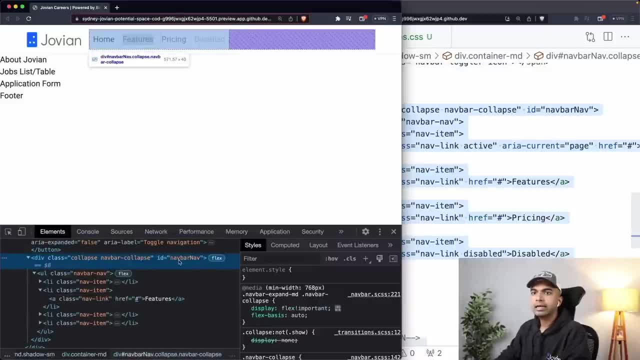 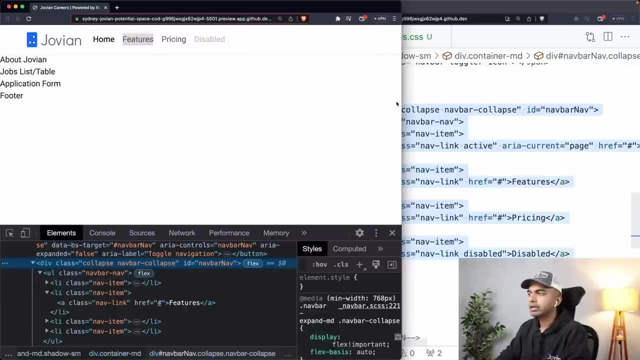 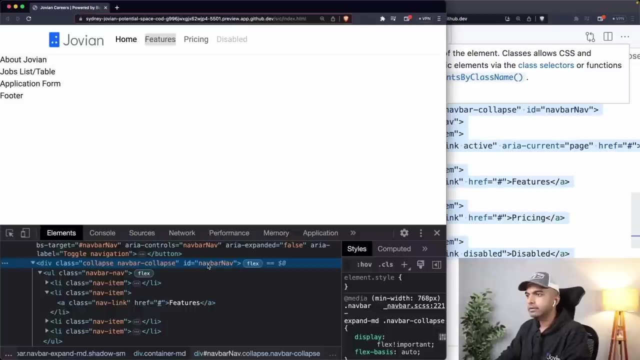 You can see that this ID Navbar nav. ID Navbar nav is visible here, But if I reduce the width a little bit, it's not going to be visible. Okay, So this is the nav. All right, This is fine. Now what do we want to do here? 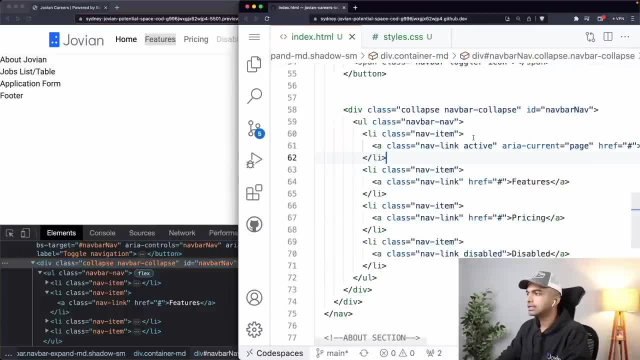 Well, we want to maybe first edit these links. So let's see, it has collapsed, Navbar collapse. I don't think there's any change we need to do here. This seems fine, ID seems fine. So I'm verifying every single line of code. 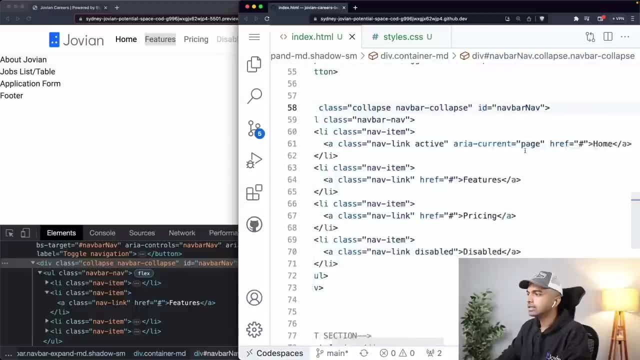 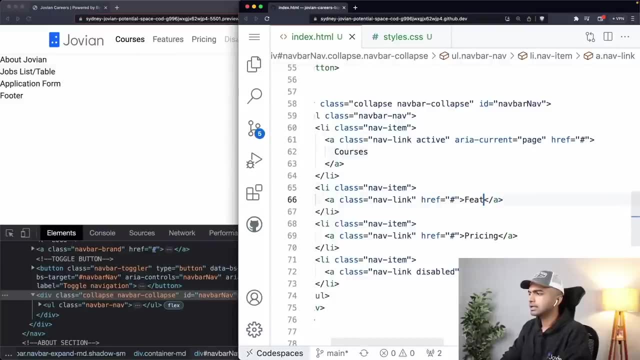 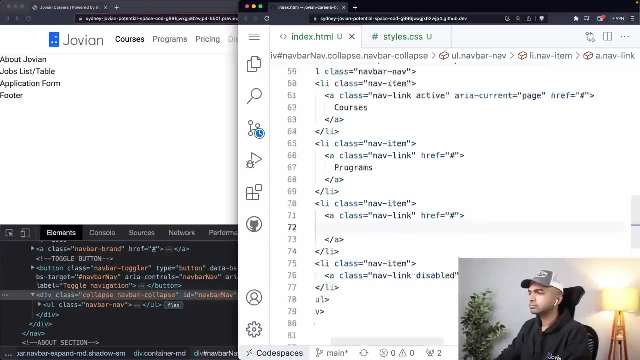 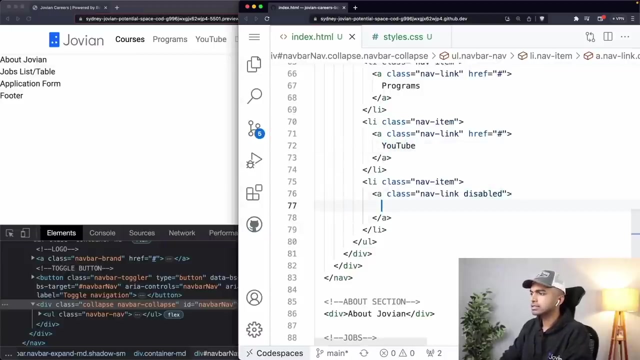 This is very important when you are working with bootstrap. Let's see, let's make the first link instead of home, Let's make the link courses and let's make this link programs. And let's make this link YouTube. And let's make this final link: sign in. 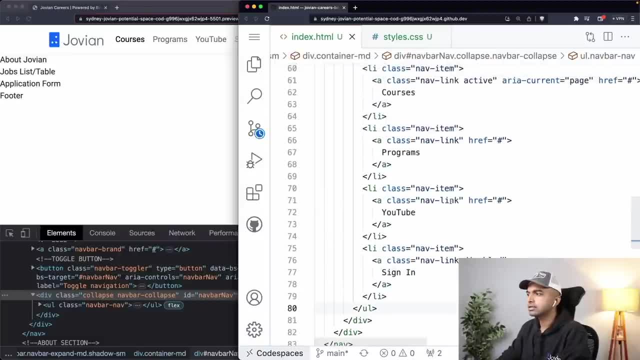 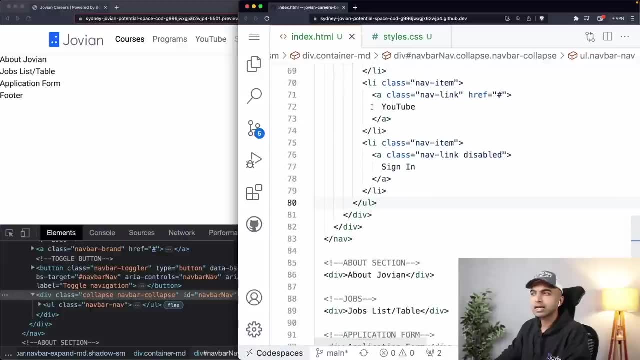 So in case somebody wants to sign in here from the careers page, They can sign in, Okay. So now, you see, now we have courses, programs, YouTube, sign in. Okay. Looking good so far. Now, of course, there are some styles that have been put in here. 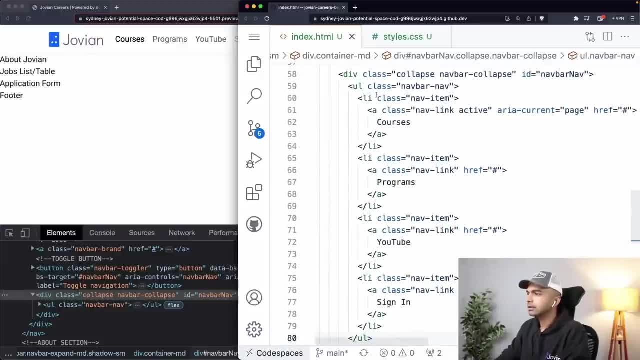 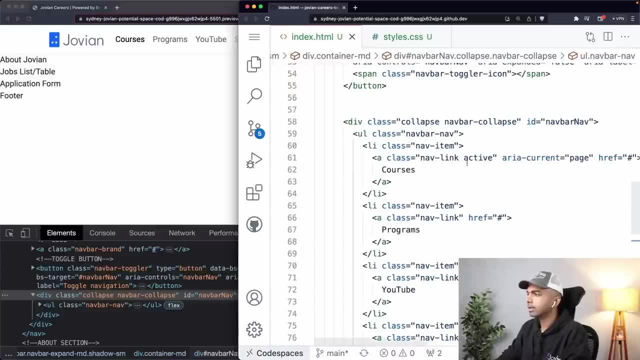 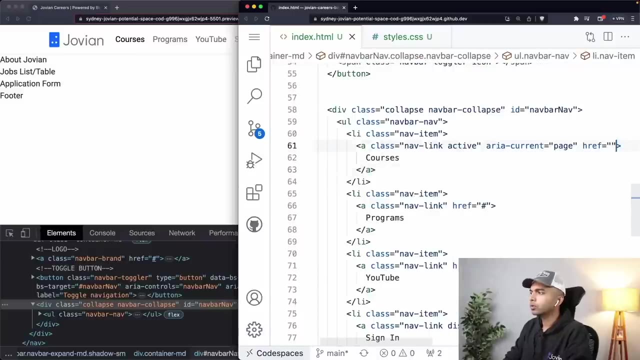 So I think I can remove those styles. Let's see, The class is nav item for all of these, And I believe we can simply change the actual hrefs first as well. Let me just set this to. Let's see: Okay. 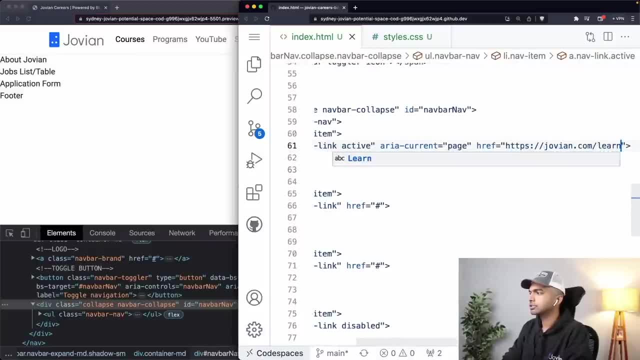 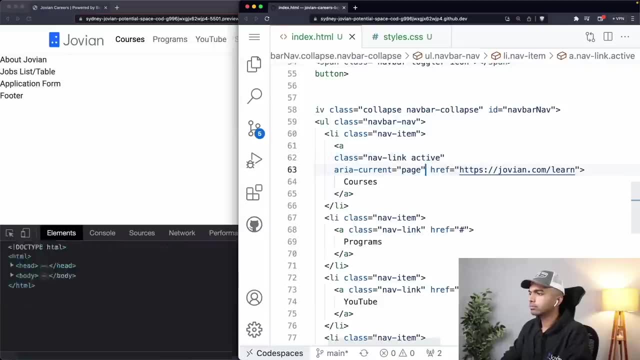 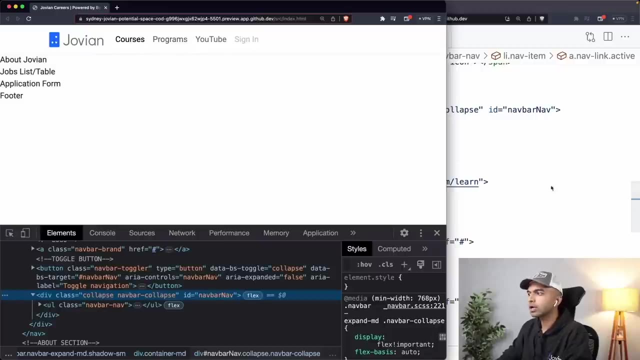 Let's see Joviancom Slash learn. So that is the link that I want the courses to go to And this is not the current page. So this current page is causing the courses to look slightly different from the programs and YouTube. 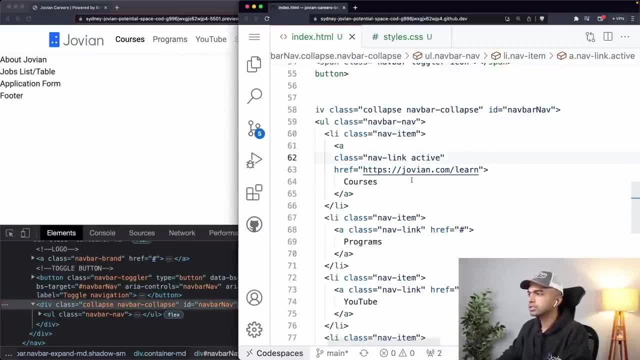 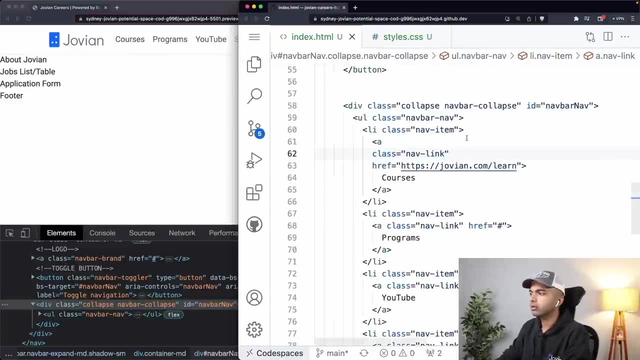 So I'm going to remove this ARIA, current, current page so that all of them look similar, And I'm going to remove this active as well, So that, Yeah, because all of these are going to some output. So when you say, active is just going to give it a special style. 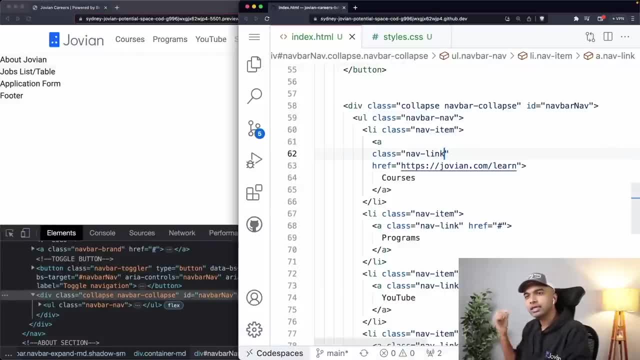 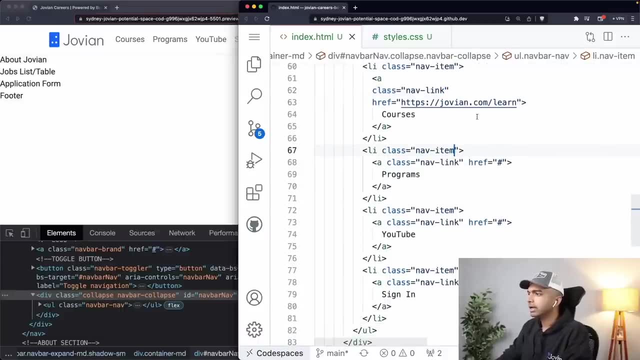 So I'm just going to remove this active as well, So you can try removing each class and see what happens, And that's a great way to understand what these classes are doing. Okay, then we have the second nav item, And I think I also wanted to open in a new tab. 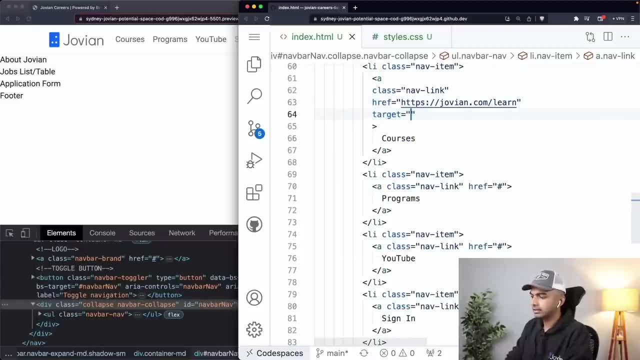 So I'm also going to say: target equals underscore blank. So now when I click on this it's actually going to open the Jovian courses in a new tab. So that is the courses nav item. Let's now fix the programs nav item as well. 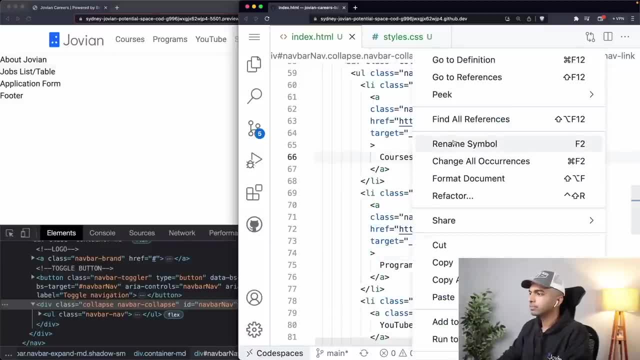 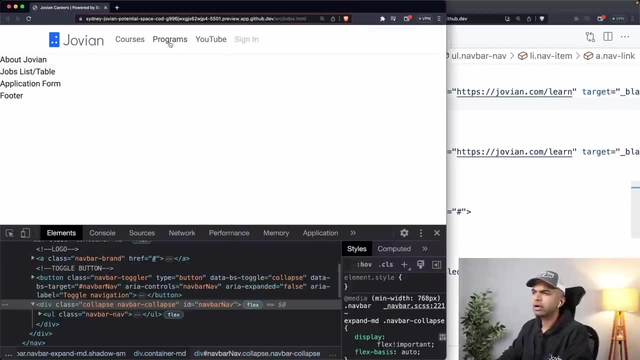 I think I'm going to send it to the same location. So we have the courses, nav item, then we have the programs, nav item. both of them are going to the same location. for now I'm. we may create separate pages later on. 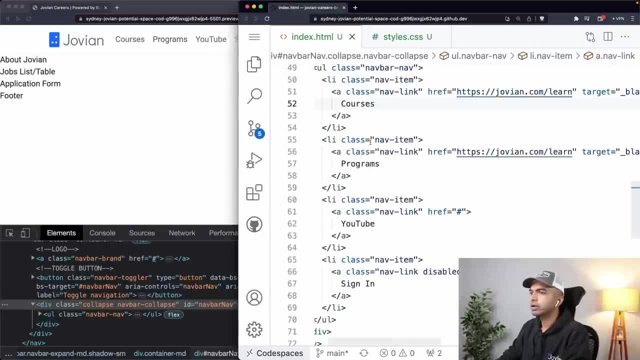 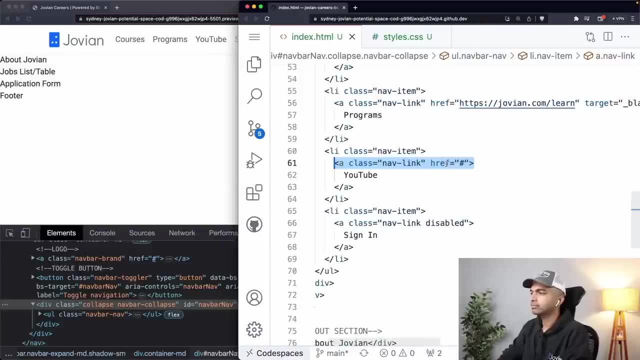 But for now both of them are going to the same same location. Okay, so these two are fine. I want to fix the YouTube link as well, So let me just copy this. Come bring it in here For YouTube. Again, it has a class nav link, it is. I'm going to give in our YouTube link here. 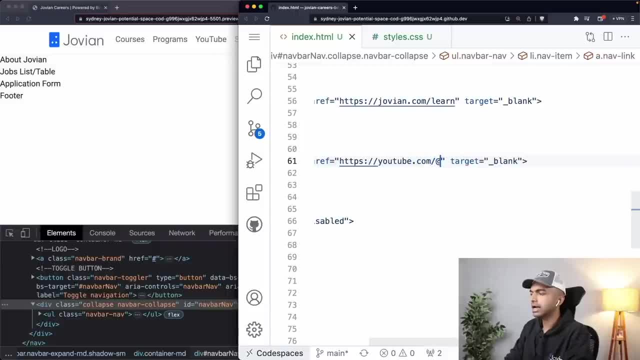 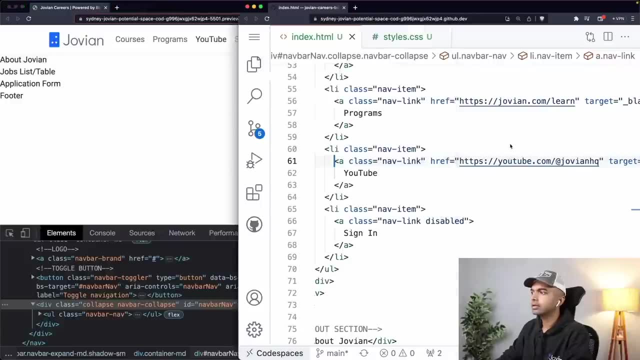 So youtubecom slash at Jovian HQ. that is going to be an YouTube link, So that is going to open our YouTube link. Perfect, And finally, there is a sign in. I want to turn the sign in into a button. 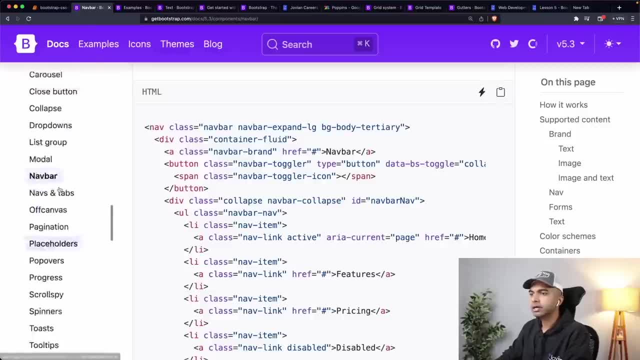 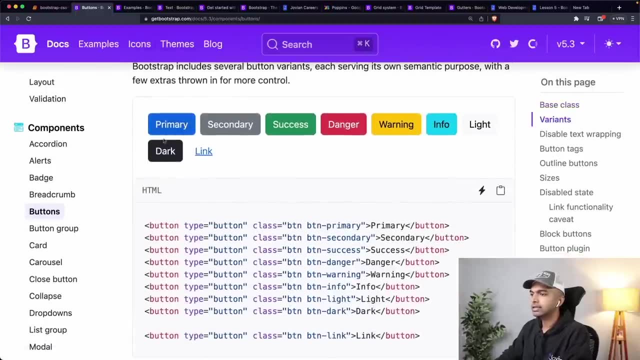 So let's come into buttons, And bootstrap also has a bunch of button classes, So let's come into buttons here. Okay, So let's come into a button simply by doing something like this, And there are like there are examples here that I all I need to do is I need to say button. 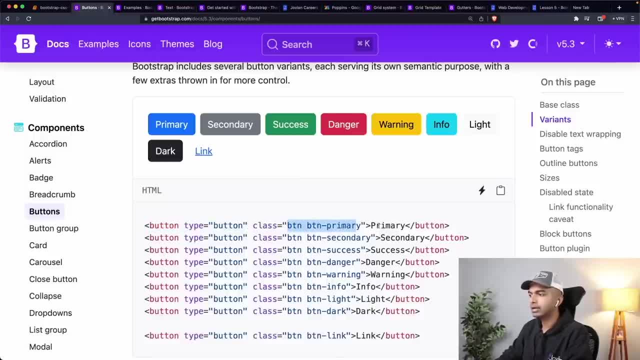 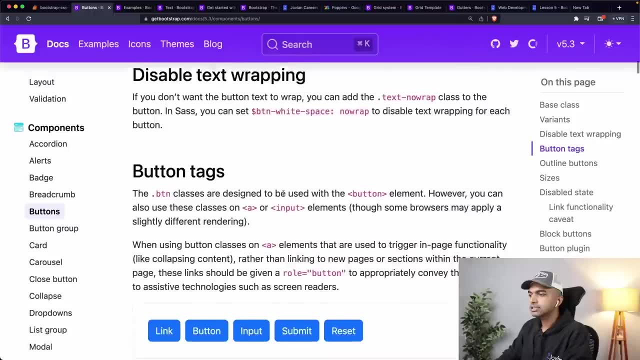 type: equals button class. equals button button primary prime. and then I can put in whatever content and this way I'm going to get this nice blue button. But one thing you can also do is you can actually just use not just a button tag, but you can. 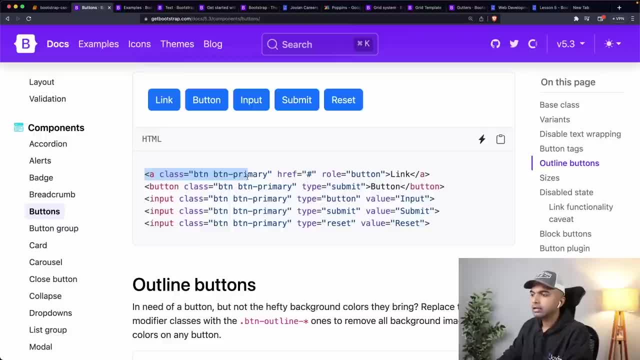 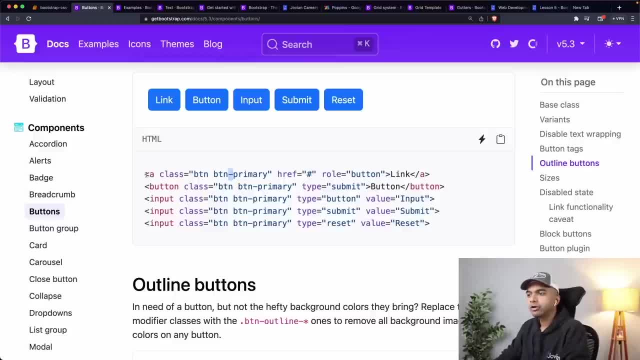 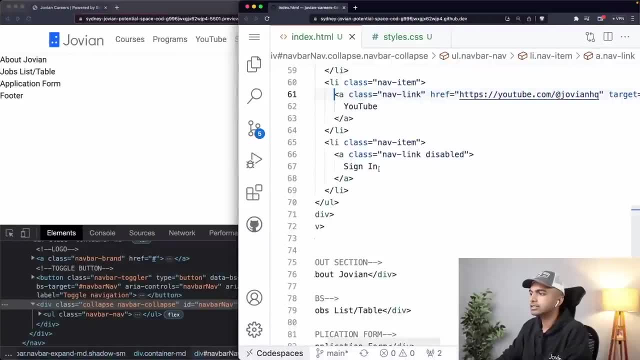 using the BTN class. Okay, so we are using a link, but we're going to turn it into a button by simply providing these classes And we can also give it the role button, just for screen readers and such. So I'm going to remove this nav link disabled class from my sign in. 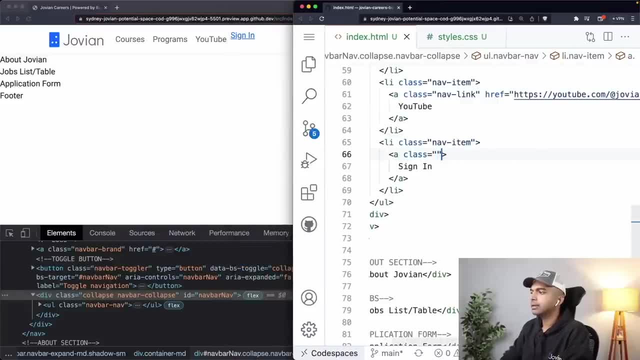 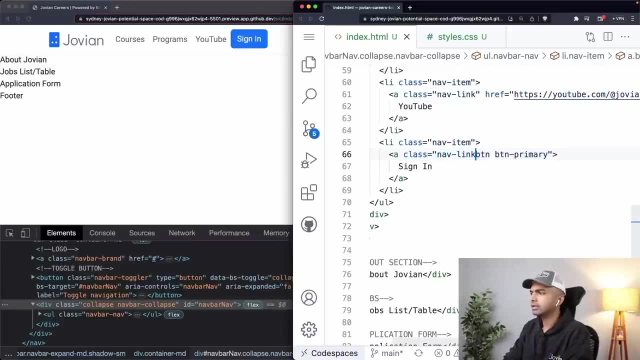 So now sign in is just a normal unstyled link And I'm going to add to it the class BTN, BTN, primary, And maybe let's see if we can also do nav link disabled class. Let's see what that does. No, that's going to change. overwrite things. 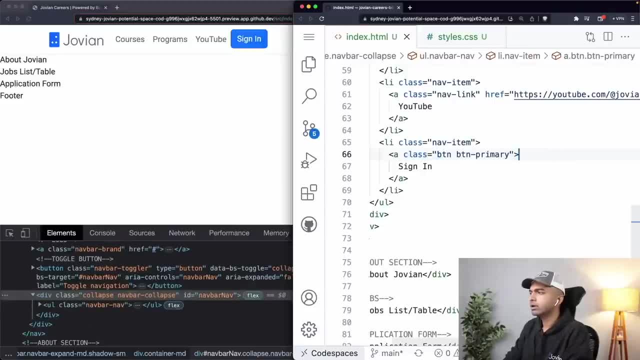 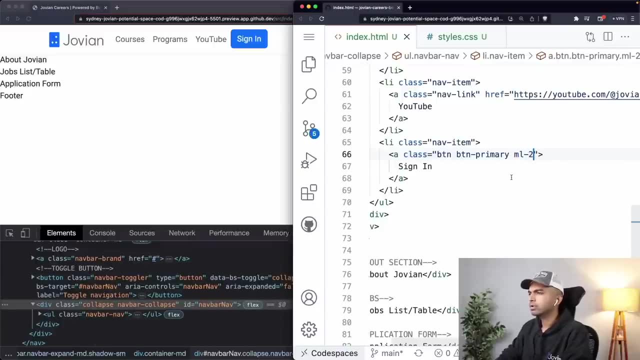 Maybe I can simply do a P L or a margin left to. that doesn't seem to be doing anything. Maybe I can do it here. I can do P X or P L, to do nothing. MX two, Yeah, MX two does the job right. 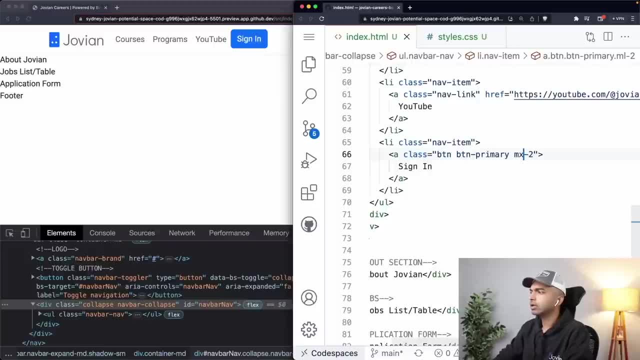 Maybe, Maybe L should also do it. Okay, I believe it is MS margin start that does the job. Yeah, So MS is margin start. So I'm just using the utility class margin start to give just some space to the button. Maybe MS three can be tried as well. 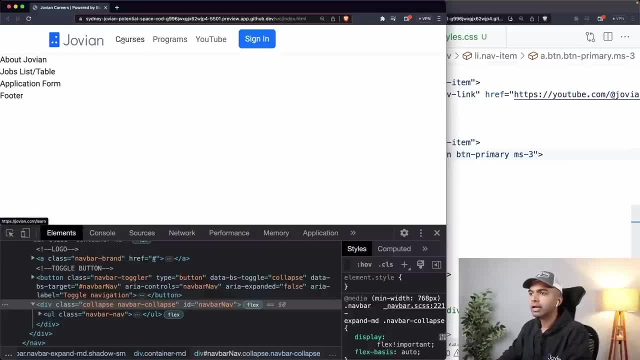 Yeah, that looks good. So now I have my Jovian logo, I have courses, programs in YouTube and I want this to go all the way to the right. I don't want it to show up here right in front And I also want it to be center aligned with the logo. 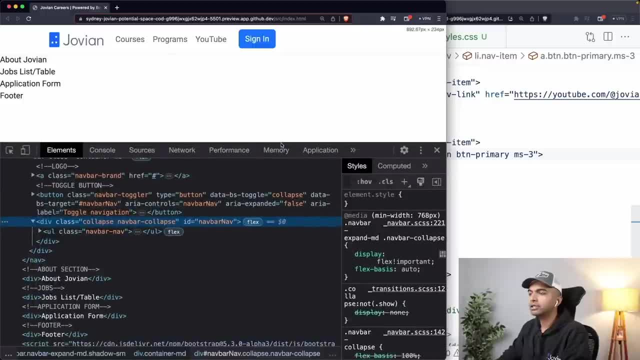 So there are a couple of things we may need to do here, and let's see how we can achieve them. Now, this is where the abstraction breaks. This is where you'll have to actually inspect the actual navbar and make some changes directly. So I am going to first just select inspect the navbar here. 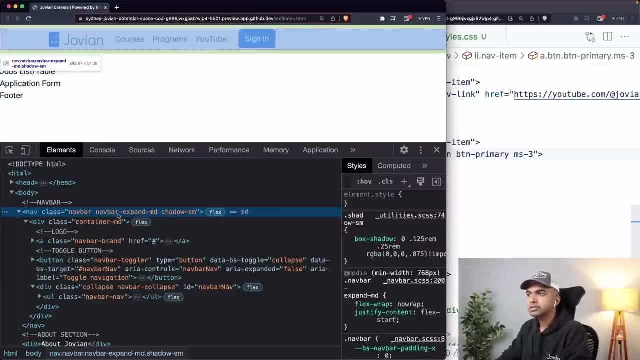 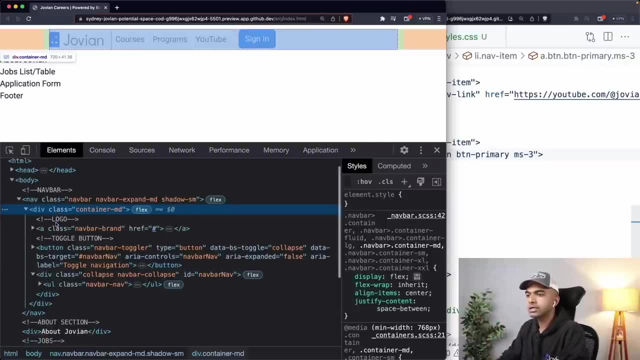 So right click, select, inspect. Okay, So this is the navbar. This is fine. And this is the container of the navbar. Okay, So this is where. this is where my entire navbar lives. This is fine. This is the navbar brand. 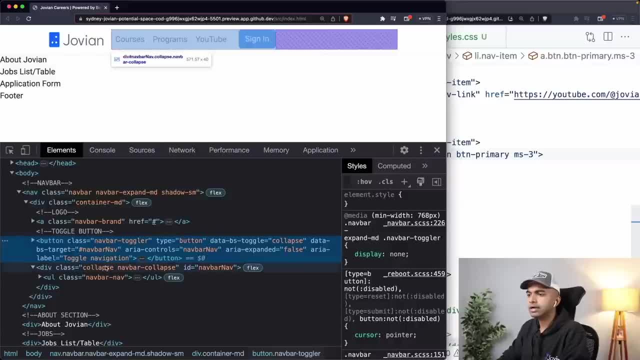 This is all well and good. Then I have the navbar toggle. that's not visible right now, And then I have this navbar collapse. Okay, So I want to looks like this navbar collapses right after the navbar brand. I want it to go all the way to the right. 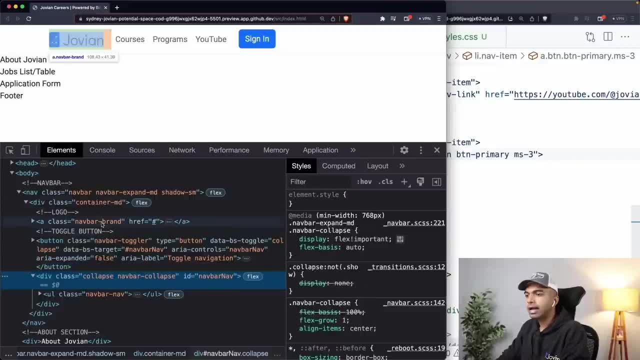 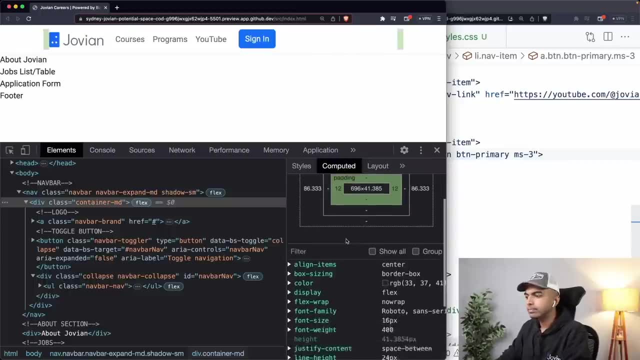 How could I do that? Let me take a quick look at the parent component, which is this container, And let me check the what is the display type of this container? Okay, So the display type of this container? the display type of this container seems to be: 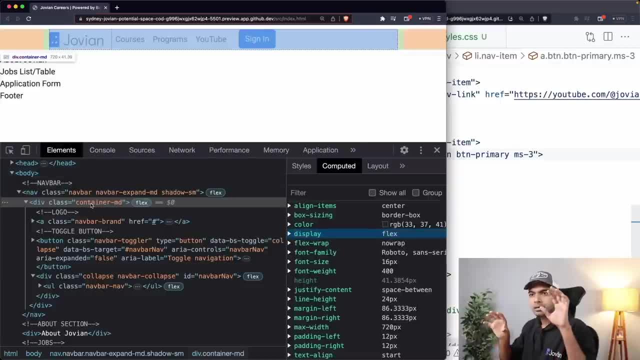 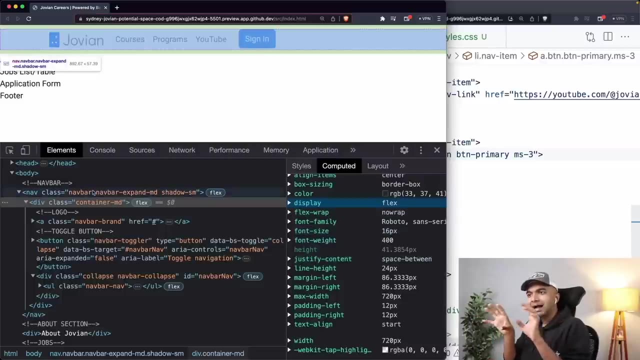 flex. Okay, So that means my navbar logo and the links are both items within a flex container And it has a flex direction row. You can verify the flex direction as well. by default it's row if it doesn't say anything. So in a flex direction row I want the contents to be spaced out. 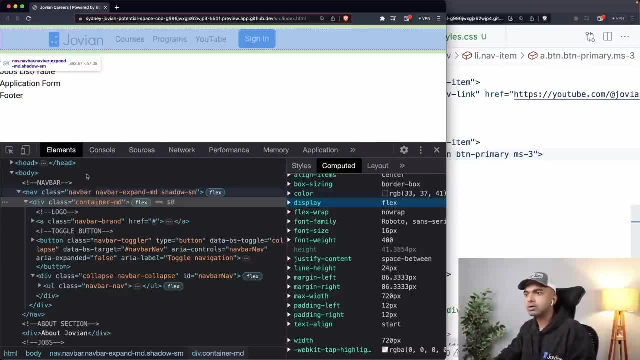 How do we achieve that? Well, along the primary axis. So, along this axis, I want there to be an automatic Space added between the starting component and the end component of the first and the second component. that can be added using justify content space between. 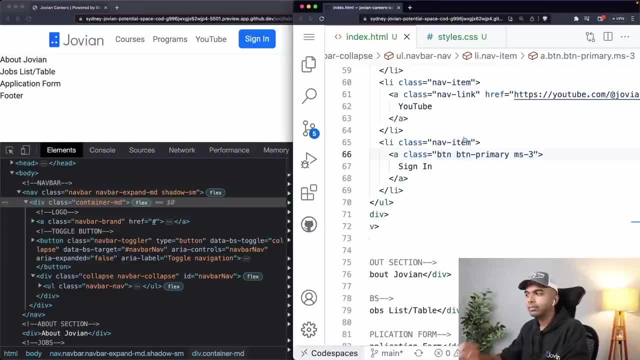 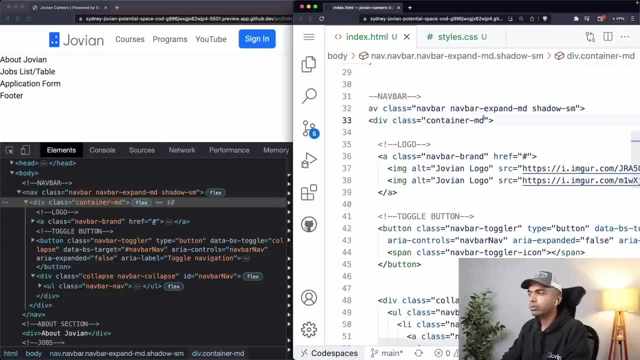 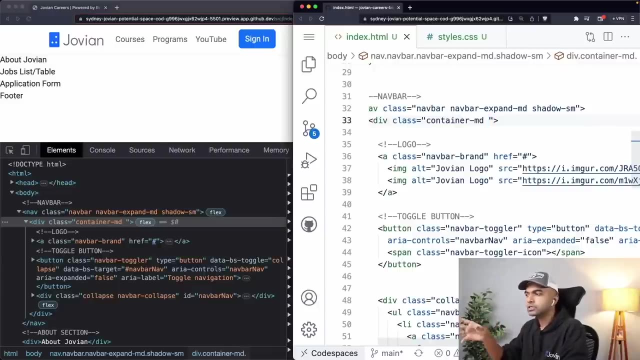 Okay. So think about this. I let you think about this, and when you practice this on your own. So what I'm going to do here is, in my container MD, which is a flex container, which contains the brand and which contains the, the list which, of course, there's, it contains a button. 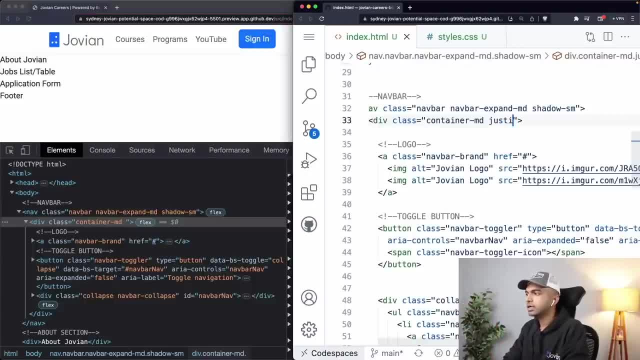 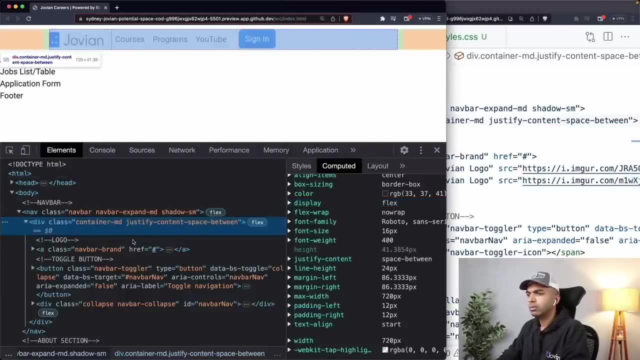 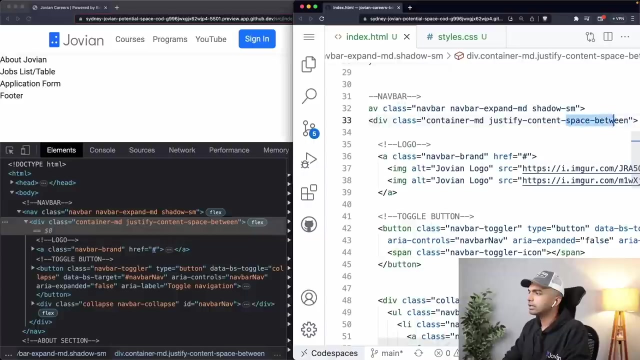 as well, which is not visible right now. I'm going to say: justify content between, or space between. what does that do? Well, that did not seems like it didn't do anything, but maybe justify content, Let's try end. Okay, That didn't do it as well. 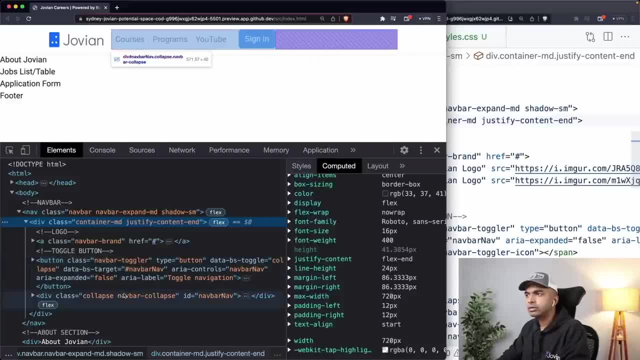 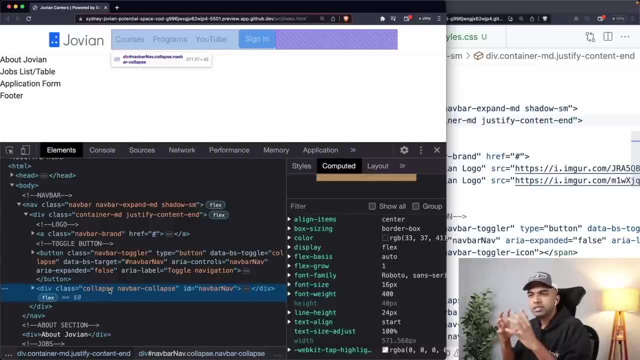 So maybe maybe I need to take another closer look at what exactly is happening here. So maybe I let me check this element. So it looks like this div is also a flex div, So maybe it's possible that this div may be taking up the entire space. 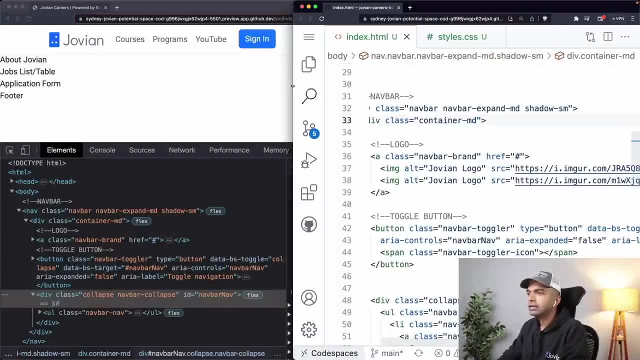 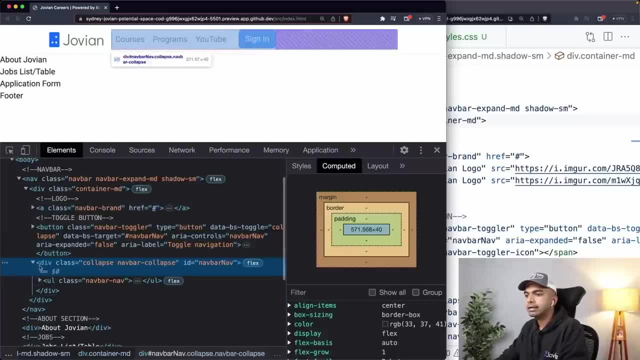 So justify content end is not working here. Let me try and come and set it on this collapse div, which is also a flex div, right? So this collapse div is also a flex container and it ha. it contains a bunch of these list items. 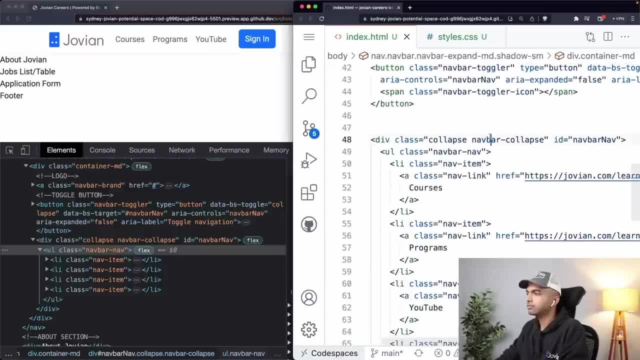 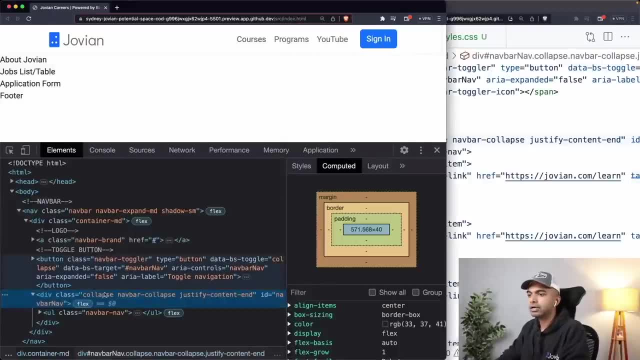 Okay, Let me define in this. So let me come into the collapse div and let me add justify content, end, and you can see that it shifted to the end. Okay, So how do I? how did I achieve this? Well, I actually just tried it out. 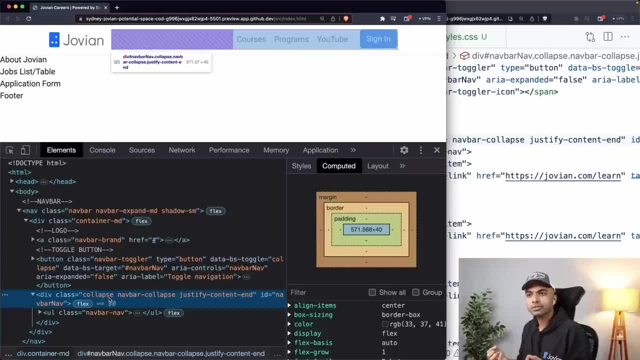 So sometimes all you have to do to achieve the desired layout is to think from first principles: Okay, This is the box I have and I need to shift something to the right or left. And how can I achieve that? using some flex property or using some display property? and 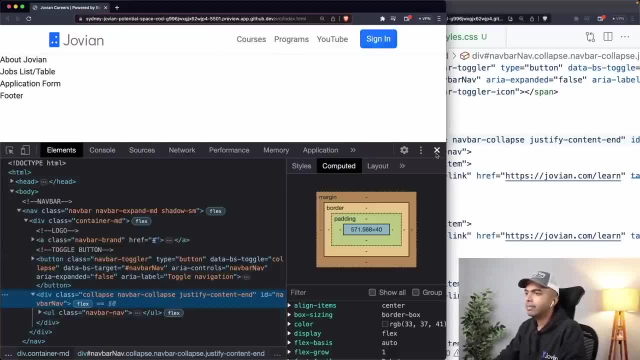 then just dig in into the inspection And fix things Right. But whenever you're using bootstrap, the one tip that I can give you right now is, if you want all of your elements in the list of nav links to shift to the right, simply go into. 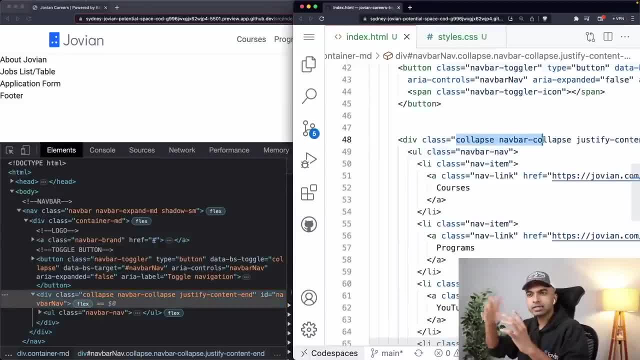 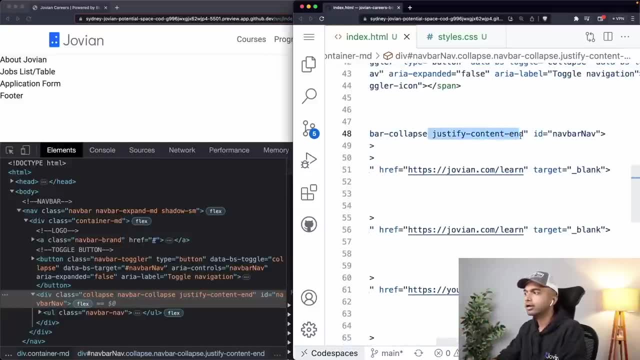 that collapse div, the collapse navbar, collapse, which is the list of things that gets collapsed at a particular breakpoint, and just start, justify content, end, and it'll shift everything to the right. Okay, And on a case by case basis, you'll just start to search this. 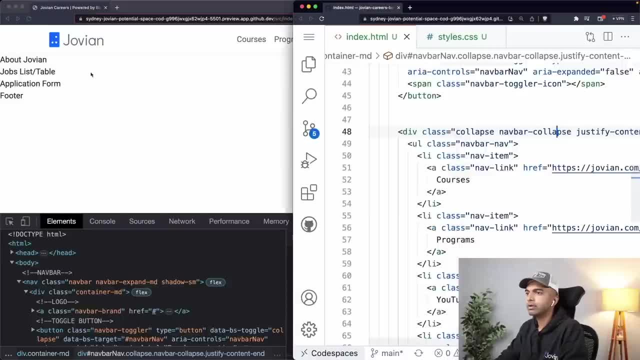 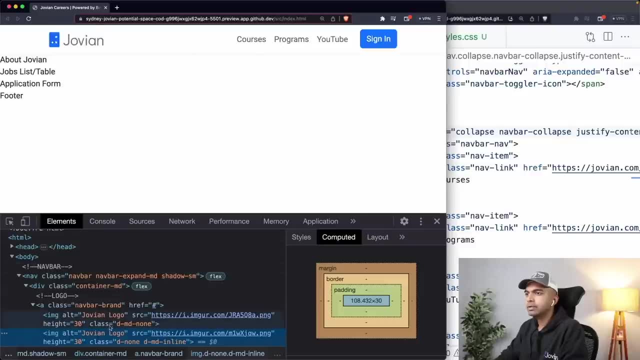 Sometimes you can just search this online as well, Okay, And you can find the answer, Okay. One other thing we can do, probably, is: maybe seems like this is not. these things are not aligned properly, So maybe I think it might also have to add an align item center here. 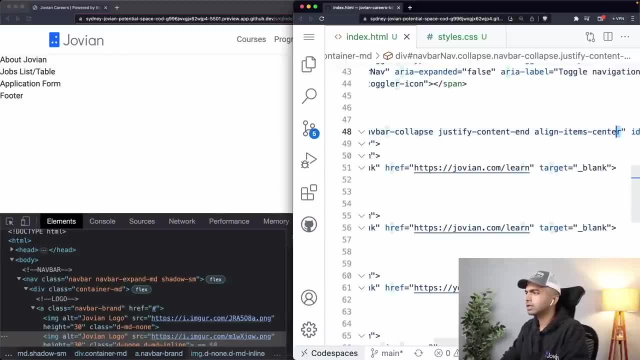 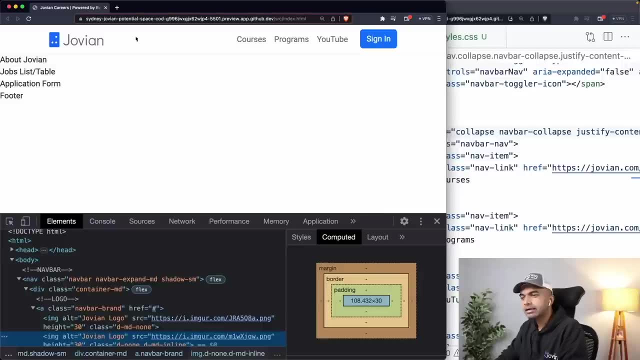 Okay, That's not doing anything. All right, I'll experiment later, but one thing I want to do is maybe just slightly fix the alignment so that courses is right, lining up properly with the center of the logo, which doesn't seem to be happening right now. 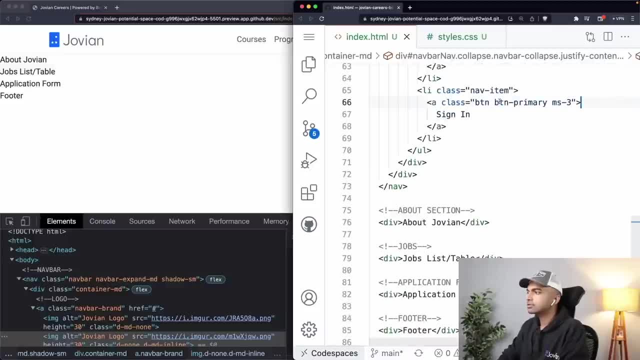 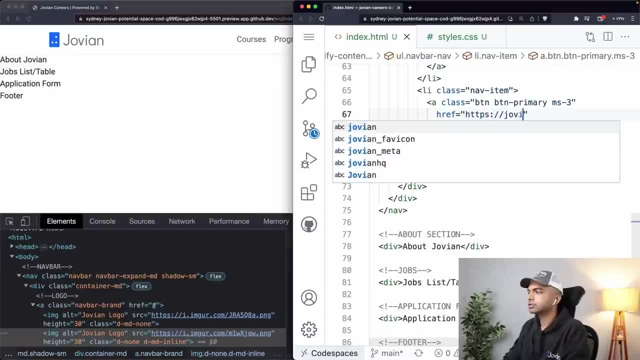 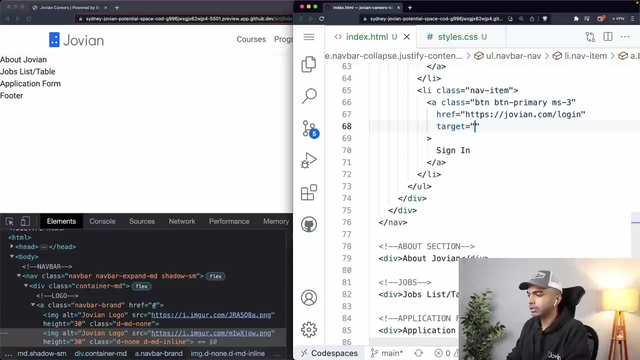 Okay, So now we have courses and we have sign in as well. for the sign in button as well, Let me just add an href and the href is simply joviancom slash login and the class or the target is underscore blank. that is simply going to open it in a new tab. 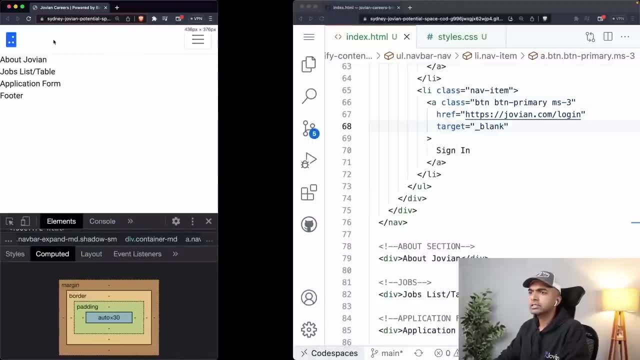 Okay, Yep, So this is looking rather nice, I would say. So here we have this mobile view. Okay, It looks like on mobile view, we need to fix the sign in button. Okay, We do not have this left. stop left padding right. 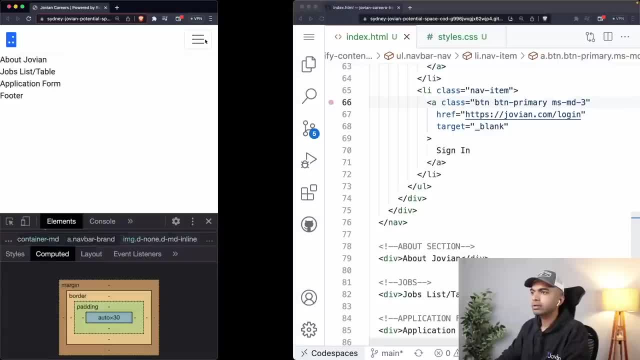 So I'm just going to trigger this from MD. Yeah, So now what's going to happen is that the margin is going to kick in only from MD. So let's see now this is looking good. I can collapse it, I can expand it. 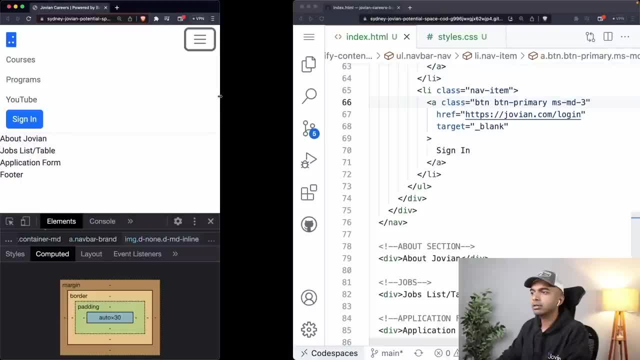 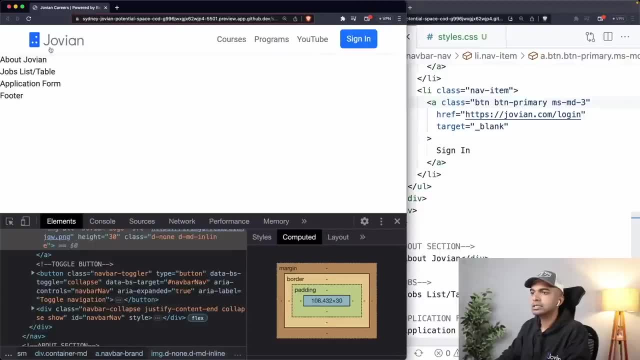 This is looking nice And as soon as I increase beyond the medium width, which is somewhere about here Now, it goes into this nice layout where I have these links Right at the top and I have this nice sign in button. I think maybe MD two might be sufficient. 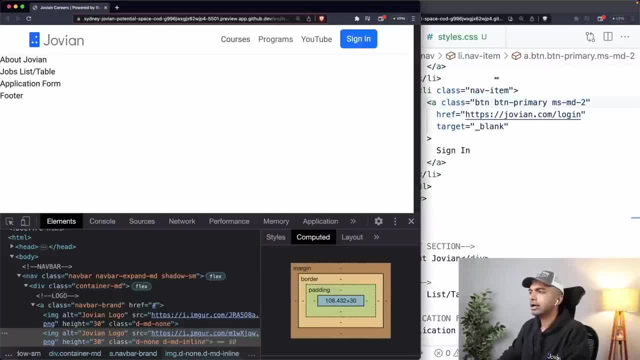 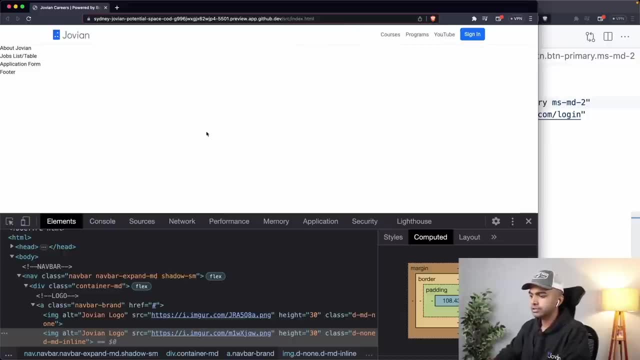 I don't really need MD three. Okay, I have this nice sign in button And this is looking pretty good. with that, we have completed the navbar. This is the original layout. I've just zoomed in a little bit so that you can see more clearly. 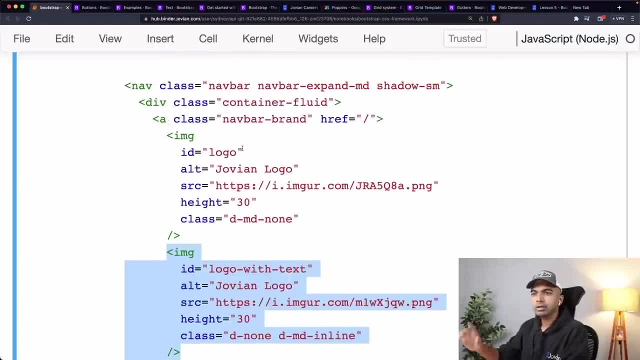 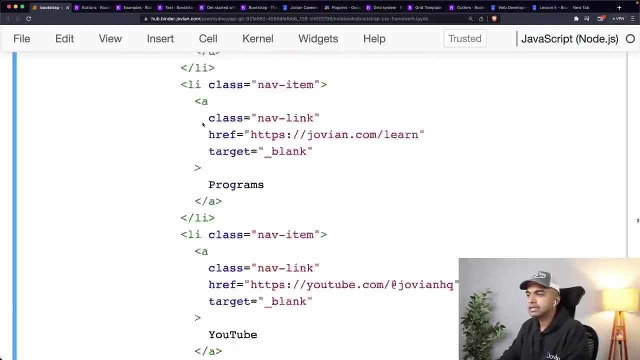 Okay, so that's what we did. You can just check out the layout exactly. the code is present here as well, But we have just made it in, made it so that it expands and it shows up a bunch of links from MD and higher right. 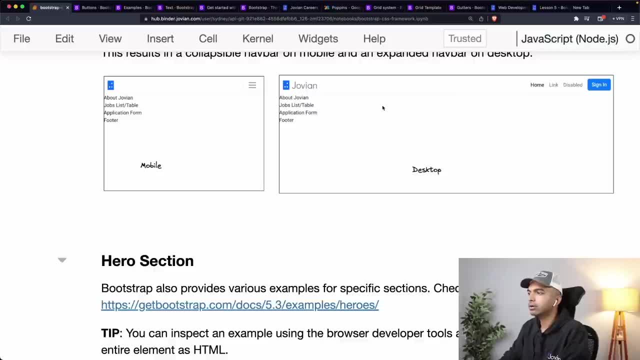 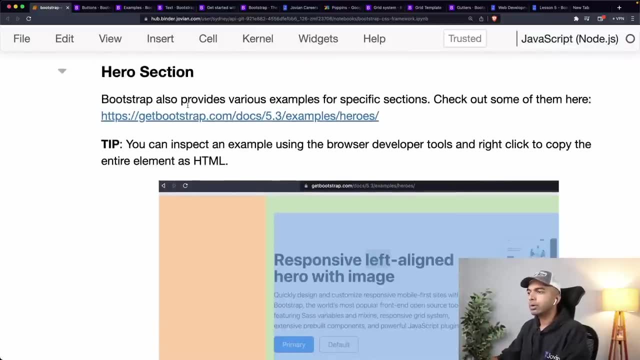 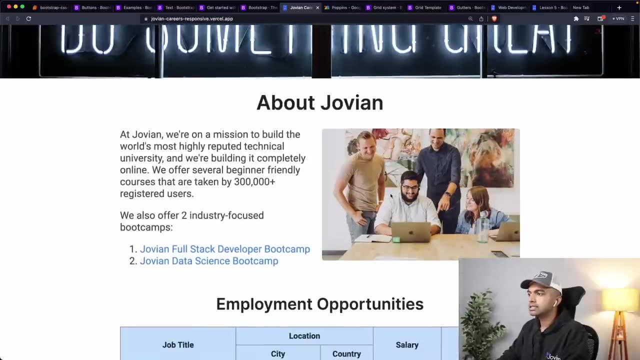 So this is the layout that we've achieved on mobile And this is the layout that we've achieved on desktop. Okay, next up is the hero section, or the about section. So this is where bootstrap also provides various examples for specific sections. But remember, in this page we have this about Jovian, then we have this, then we have this. 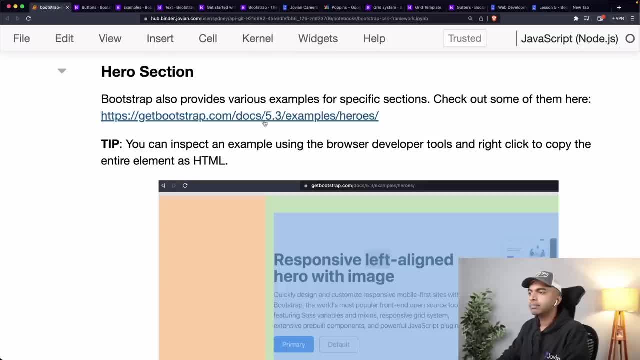 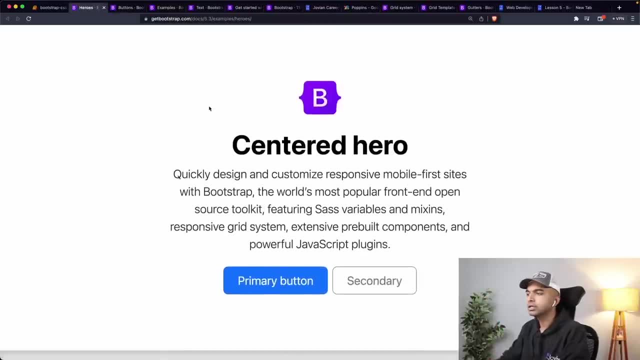 and then we have this banner image as well. Let's look at some examples from the bootstrap examples. So these are all. these are a bunch of examples for the hero or the about section And for this looks like there is this centered option that we can just have some centered. 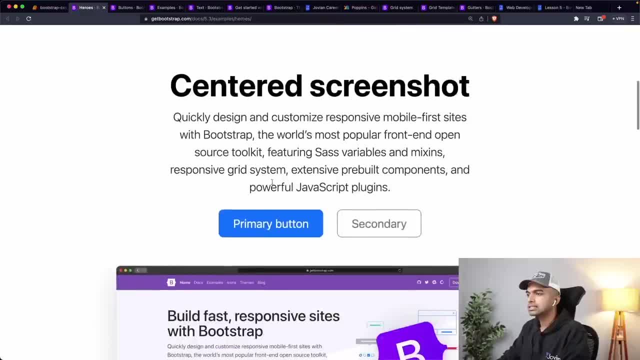 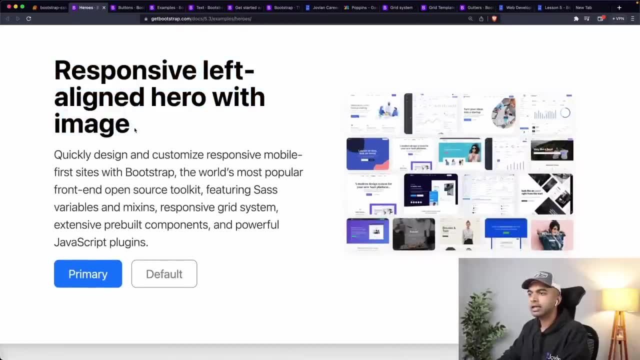 content on the page. I don't want that. There is this center option with an image below it. That's not what I want either. Okay, this looks promising, So I have some text here. I have some text here, and then I have an image here that looks. 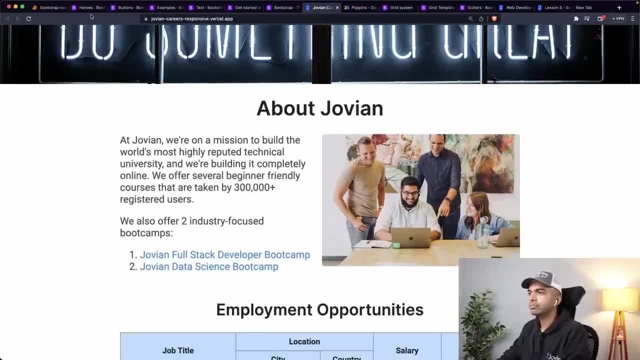 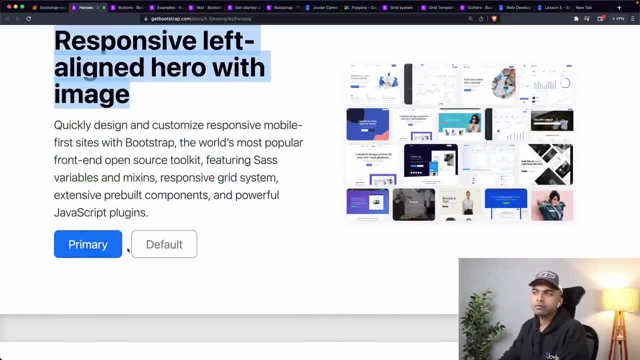 somewhat similar to what I need here. okay, text, image, etc. And maybe this layout is actually better, where the text, even the title, is on the left and not on the center, And then I have these buttons Here, but I don't have to use these buttons. instead of these buttons, I can simply put. 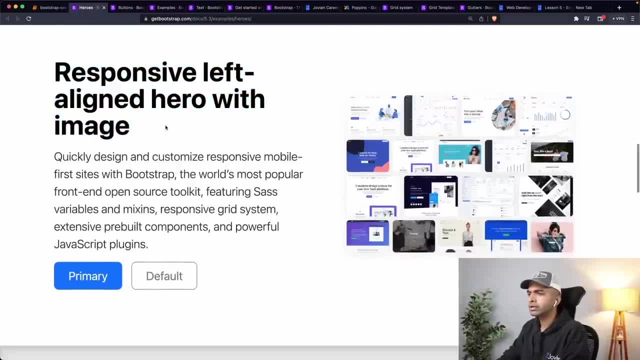 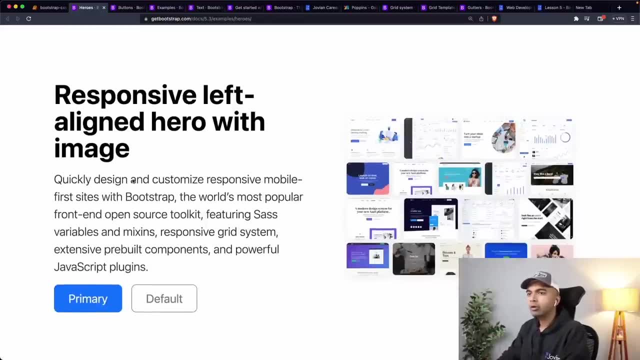 in these two items that I have here. Okay, so I guess I'm going to use this layout And this is one of the examples. on this examples page we have a bunch of examples. How do I get the code for just this example? there is a way you can download the code and 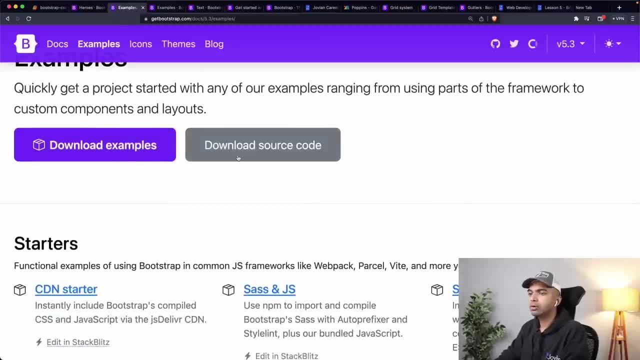 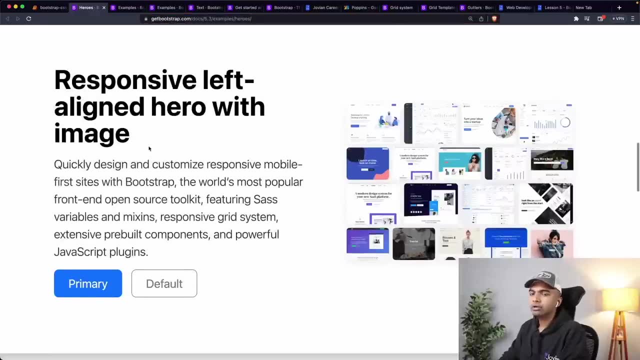 then search it So you can go into bootstrap examples, you can download the source code of these examples, you can open the hero folder, etc. etc. But I'm going to show you a quick way When you're looking at a bootstrap example. 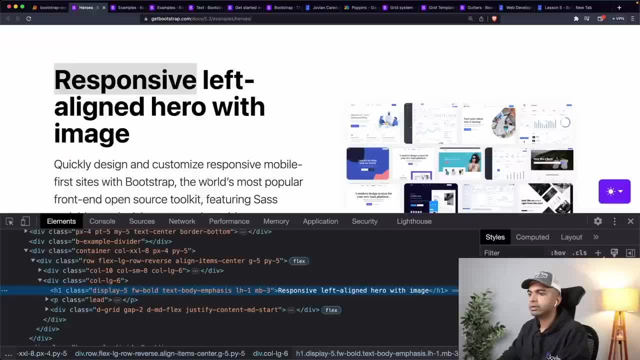 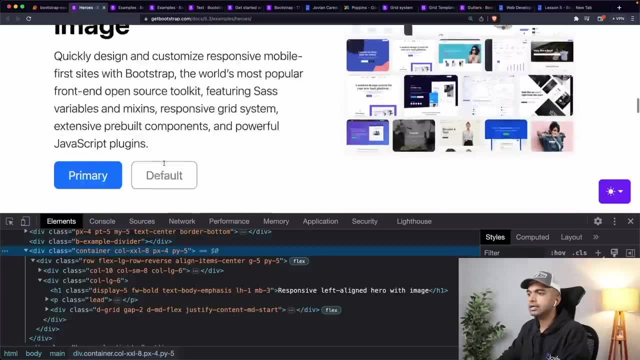 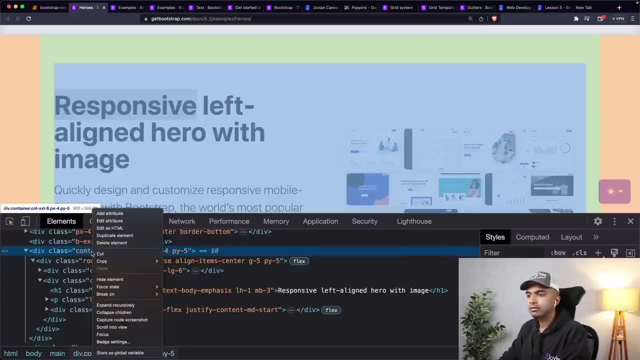 Just right click, click, inspect and find the outermost container. So okay, this is the container and looks like this container contains this entire hero element inside. it is the entire thing. So you can just click on this container, right click, select copy element. 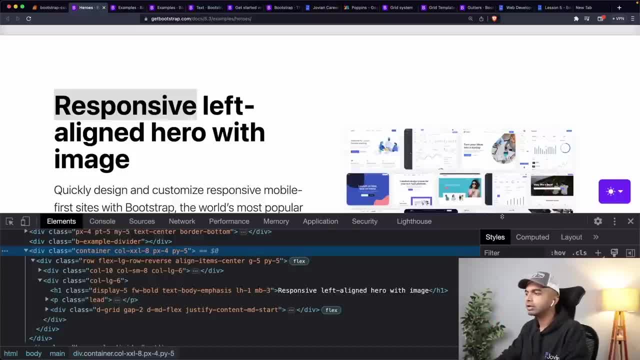 And that is going to copy the HTML code for this entire container that we're looking at here. Okay, So with one click I've copied the entire HTML code for this container, And now I'm going to copy the HTML code for this entire container that we're looking at. 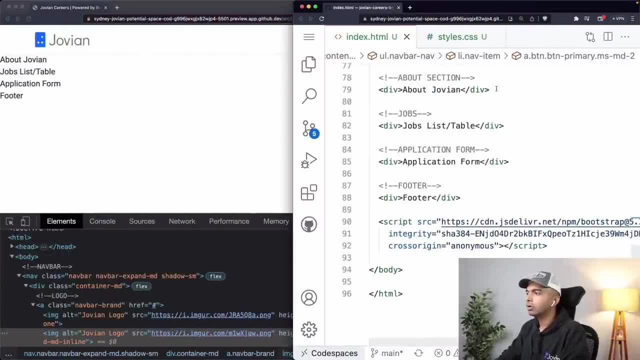 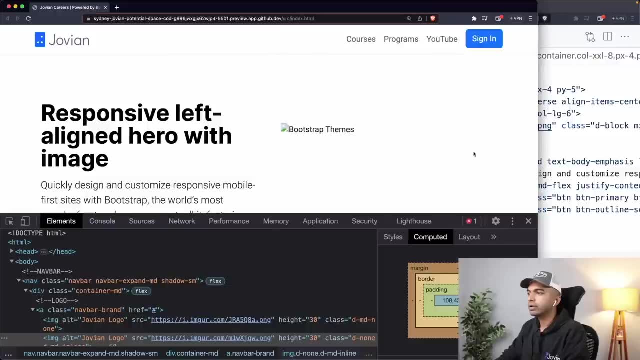 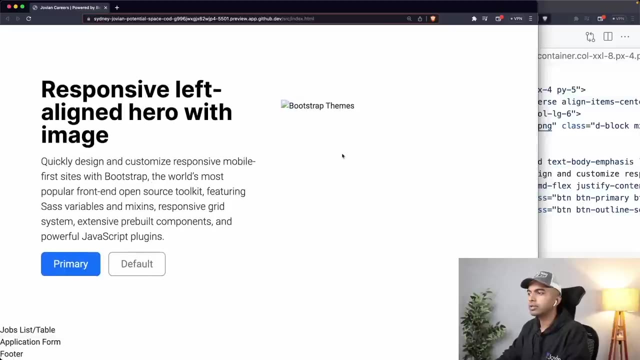 here And now I can come in into my code And here in this about Jovian section, I'm removing whatever placeholder text I have. I'm just going to paste in this container And just like that you can see that we got this nice responsive left aligned hero with. 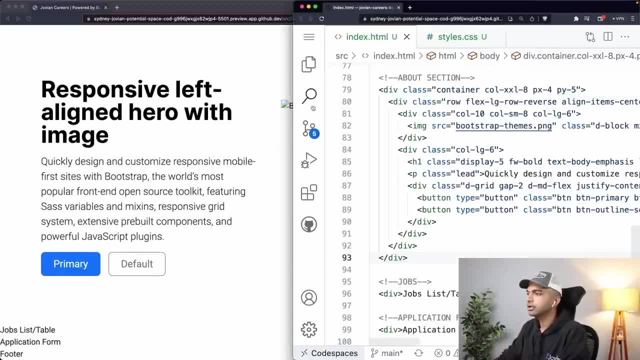 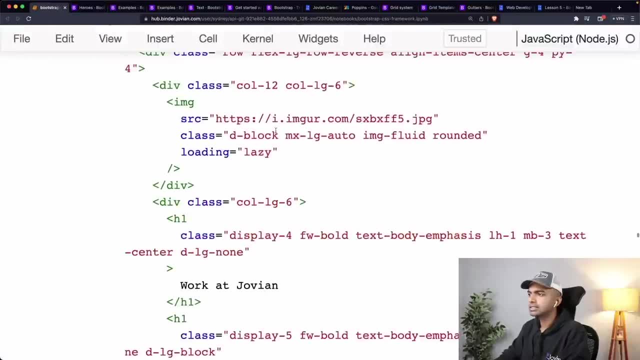 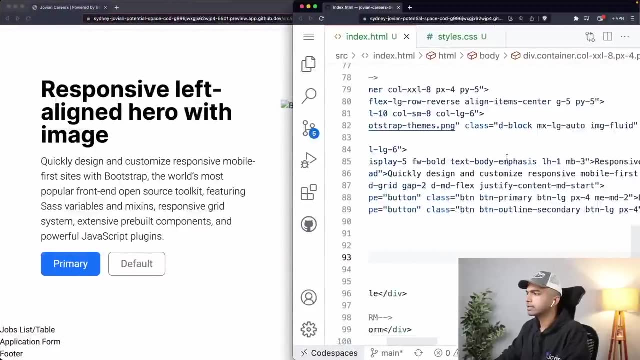 image And, of course, the image is not present here, So we can change this image. we have an image here. actually, I think we have a link to an image here that we can grab. Let's see. Yeah, So I've. I've hosted this image online so that I can just copy it over easily. 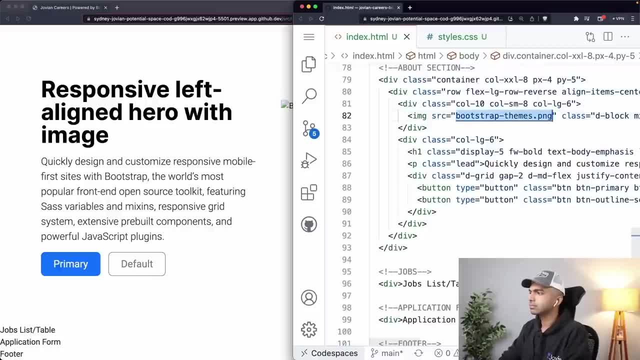 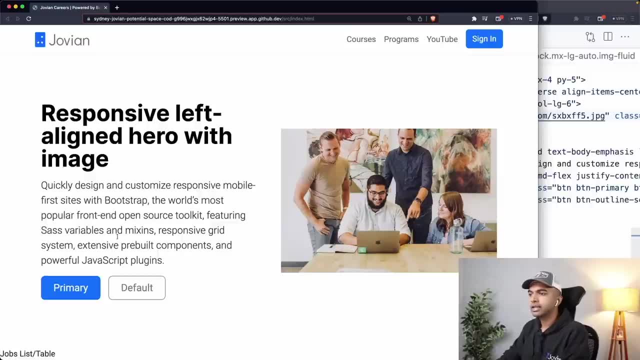 Let's see, I am Yeah, so the image source is this. Yeah, And so with that I have this nice layout where I have this responsive left aligned hero with image and with some text, with these buttons, and I have this nice image on the. 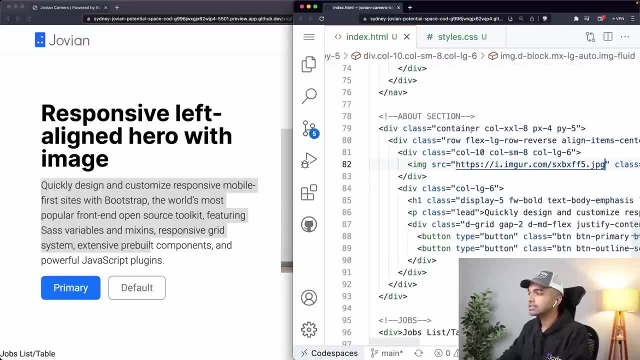 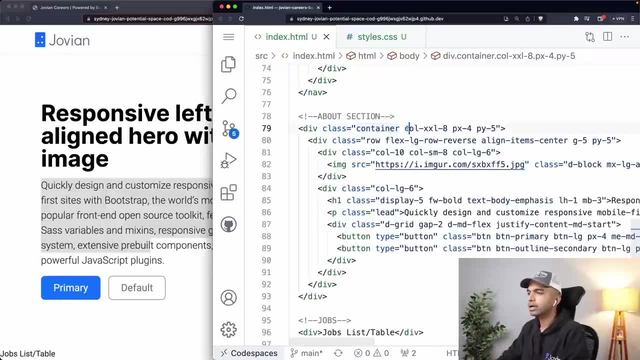 right. Okay, looking pretty good, And let us start understanding and customizing this. Okay. first thing, I wanted this to be a container. I think that's fine. I want the content to be centered on the page, no matter what screen size we are on. 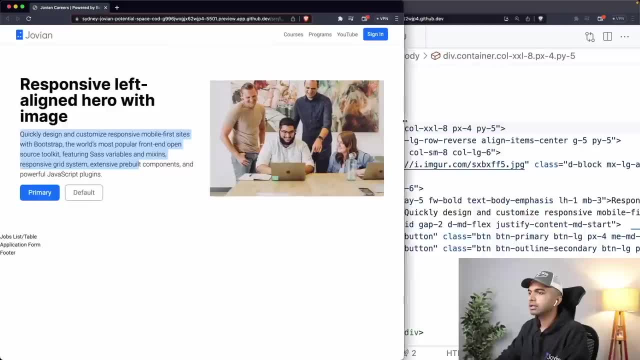 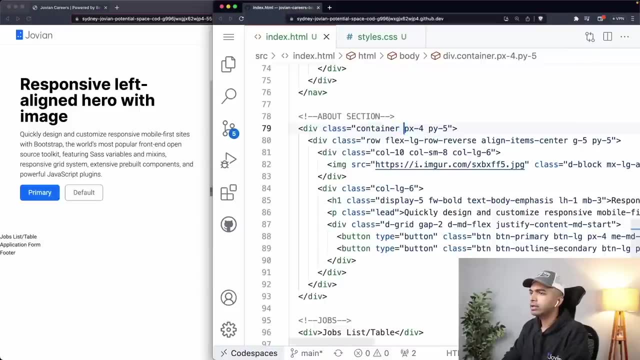 So this is fine. It's. this content is always centered on the page. Okay, let me get rid of this. I think I don't need this call XXL eight. I am not interested in that right now. It has this PX four. what is this PX four? 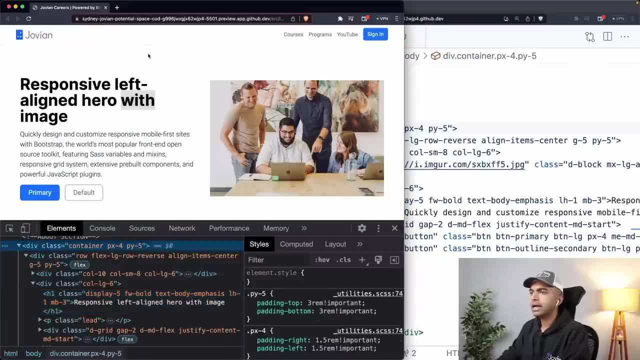 Okay, so this PX four seems to be this padding on on the left and right. Okay, I think I can keep the PX four. It also has this PY five, which is the, Which is the space above it. I think maybe this PY five may not be necessary right now. 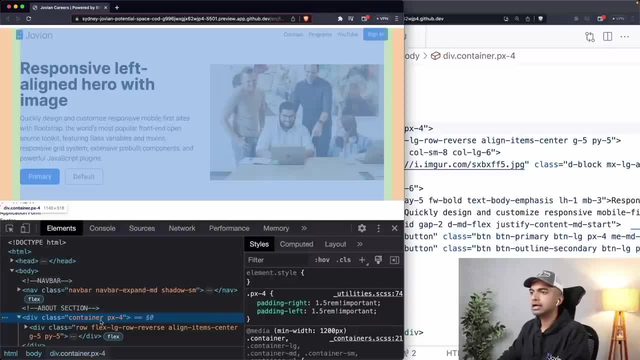 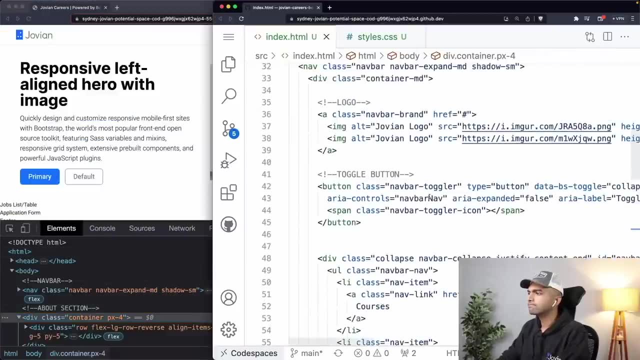 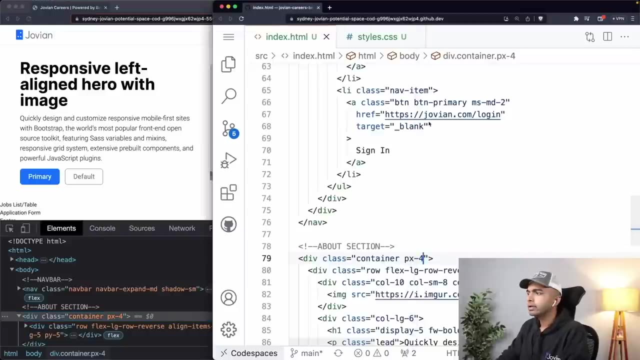 So I'm going to get rid of this PY five and automatically you can see that the top and bottom padding has completely gone away. Right Yeah, So that is looking good so far. Next, let us come in here and let us check. 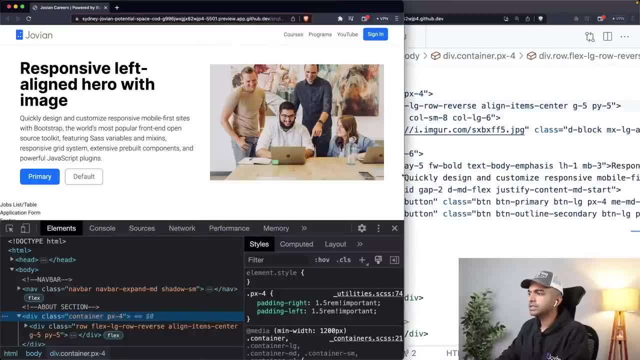 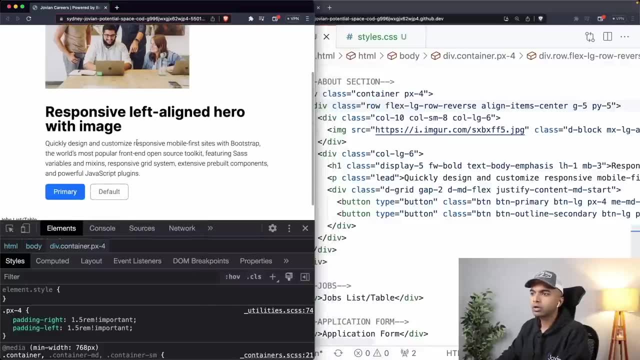 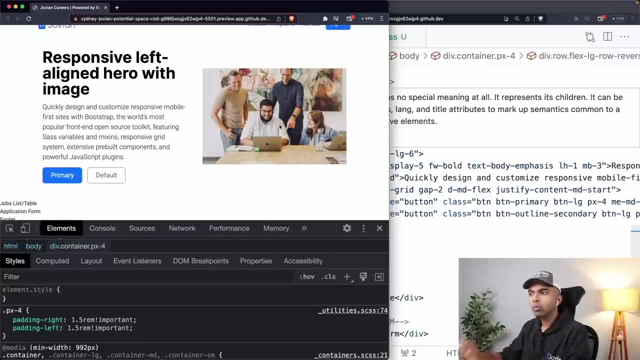 Okay, what's happening here? So it looks like we have flex By default. we have, like it's just a normal div with things going top to bottom. That's fine, And at some point it becomes a flex container with the direction row but not just row. 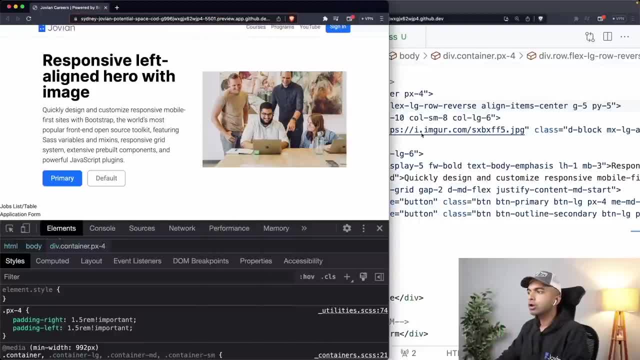 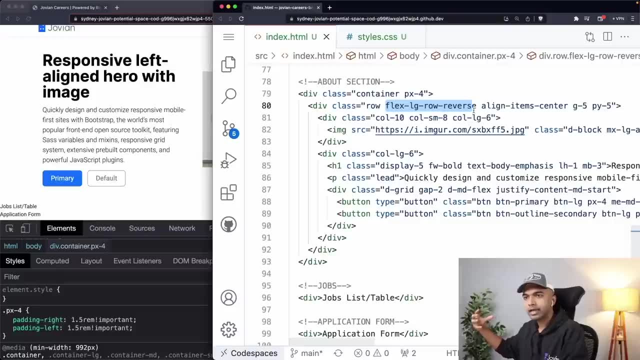 it becomes a flex container with row reverse. So on large screens we have flex LG row reverse, which means on large screens it becomes a flex container with a direction row reverse, And that is why the image comes on the left And the. 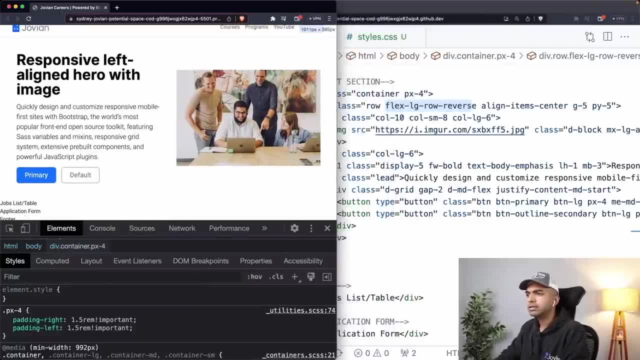 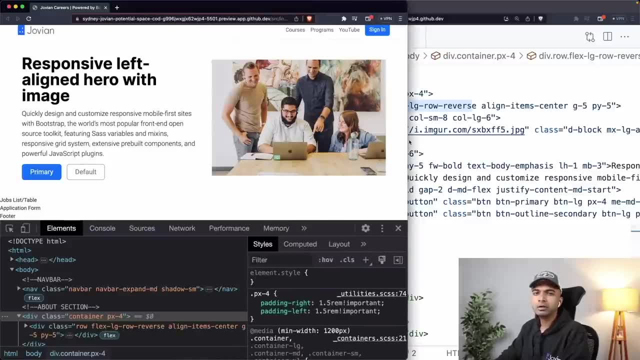 On the right And the text comes on the left. Okay, I think that works for me, that I have this top to bottom layout here. This is fine. And then I have this left to right layout here. This is fine. I may need to do some centering, but it's fine. 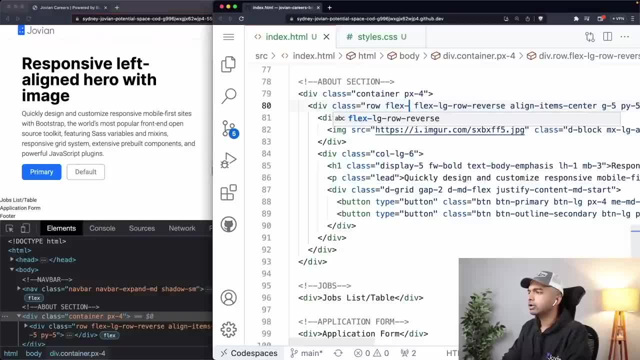 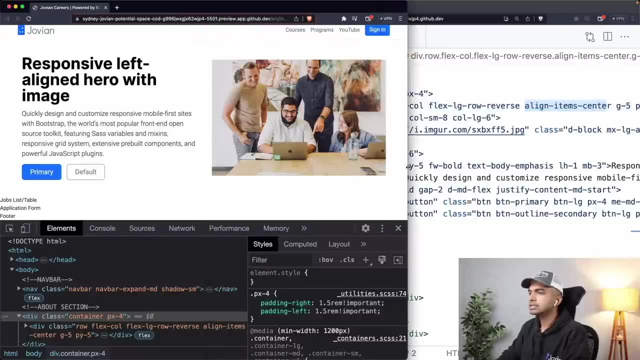 Okay, Maybe I can just use a flex call layout, initially a flex column layout, so that there's already this align item center. So what that can do for me is just make sure that the content becomes centered. Okay, That's not exactly. 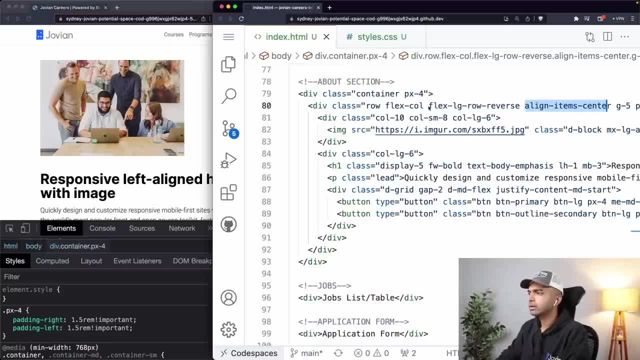 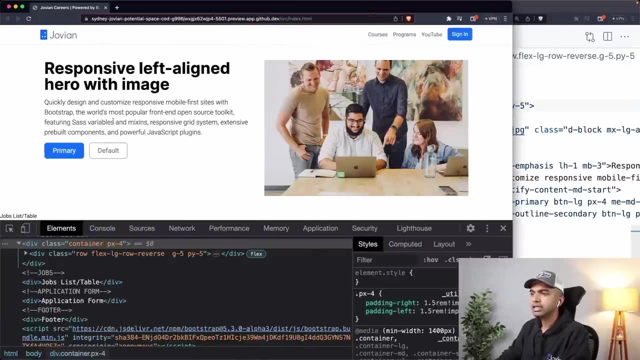 Doesn't exactly Happening yet. Okay, Maybe we don't need this flex call here. So this is okay. Align item center. I think what this does. I can remove it and see what happens. So when I have align items, when I don't have align item center, the text comes on the top. 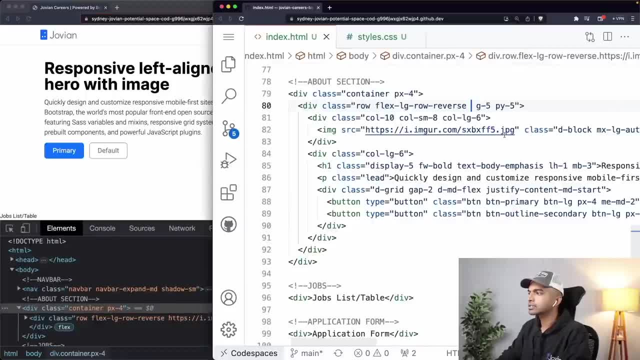 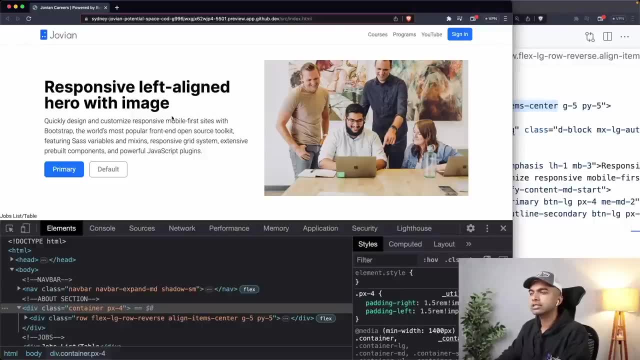 and it is aligned with the top of the image. When I have align items- oops, when I have align item center, the text is center, aligned vertically with respect to the image. Okay, Earlier it was here. I think I like this better. 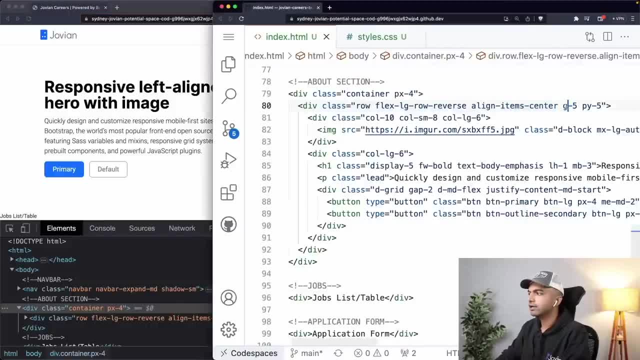 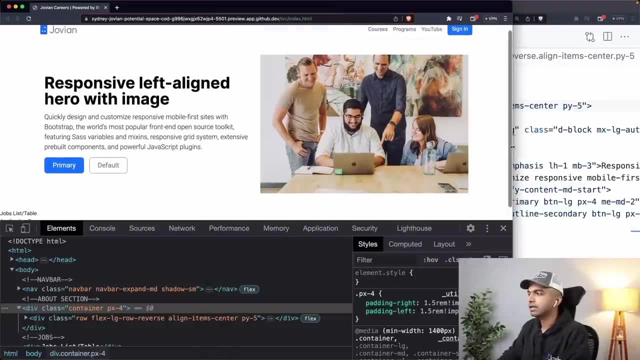 So I'm going to keep align item center. Okay, There is this G5.. Let's see what happens if we remove the G5,. well, it looks like there was some shift in the gaps. I think it's fine. It's probably okay. 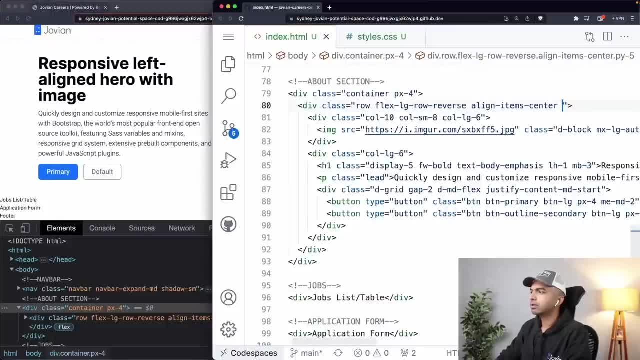 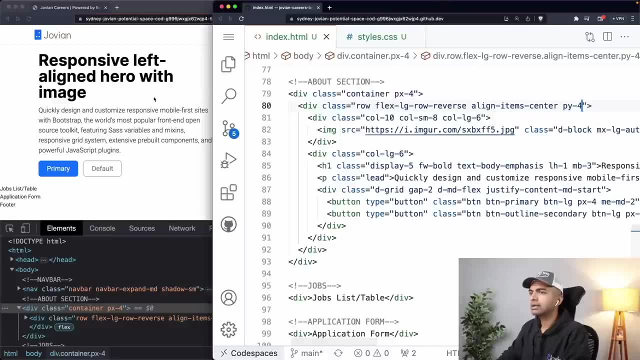 Not a big issue. There is this PY5.. Okay, Do we need this PY5?? Yeah, I think we need that PY5.. Maybe I can just make it PY4.. Maybe we don't need that much space. Okay, Looks fine. 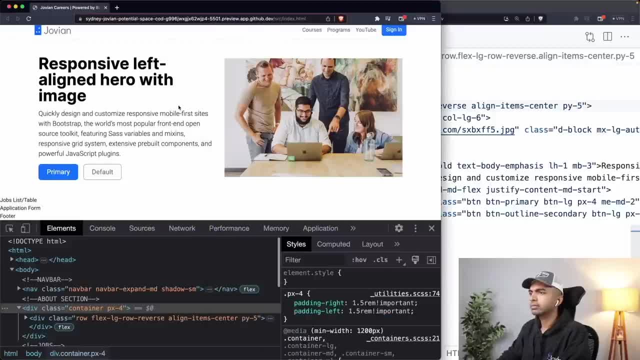 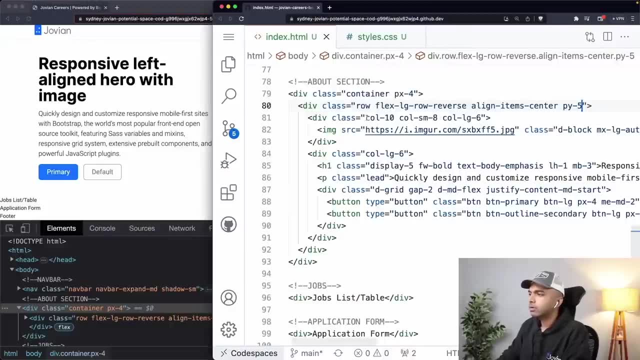 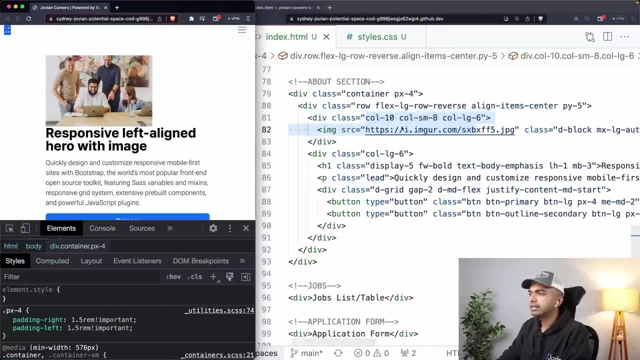 PY5 is fine too. Okay, Looks fine. So far, my layout is looking good. Then we have this image. So we have this call 10, call SM8, call LG6, a bunch of stuff going on here. I think I'm going to make it very, very simple. 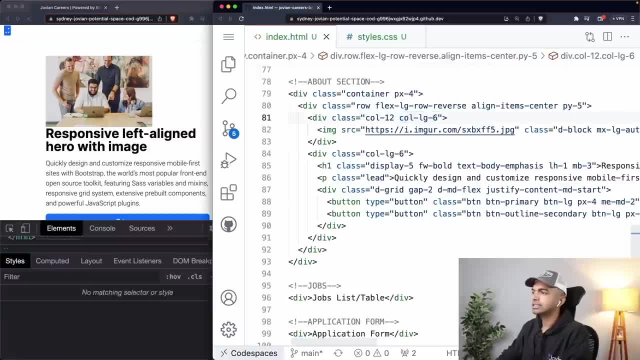 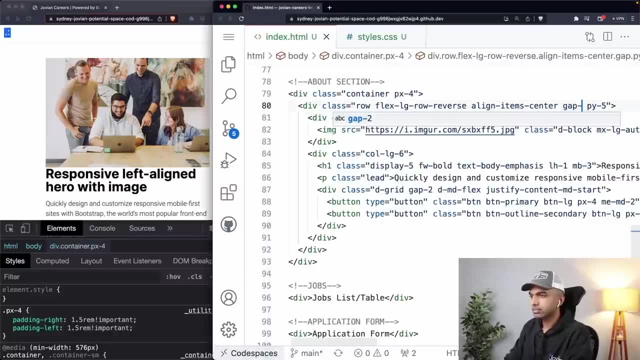 I'm just going to say: call 12 and call LG6 so that it takes up the full width, And I think we'll probably need that gap five now because, yeah, I think we need that gap. Maybe I can make that gap smaller. 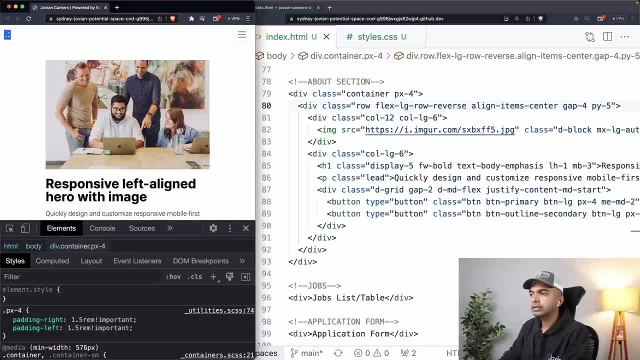 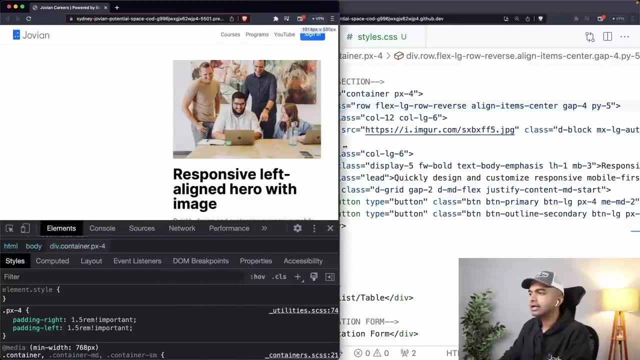 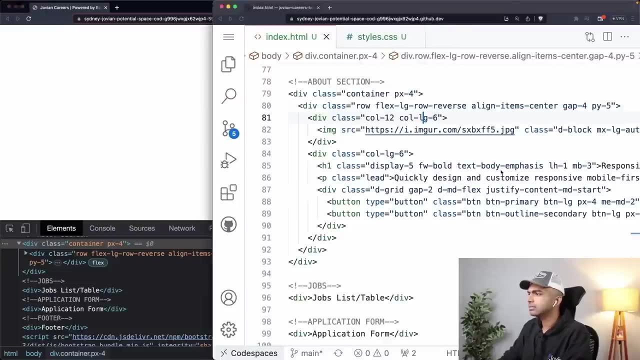 Yeah, So I wanted to take up the full width, the div containing the image. I wanted to take up the full width on all screens And then at some point I wanted to take up just half the width. So at LG I wanted to take up half the width, but that doesn't seem to be happening. 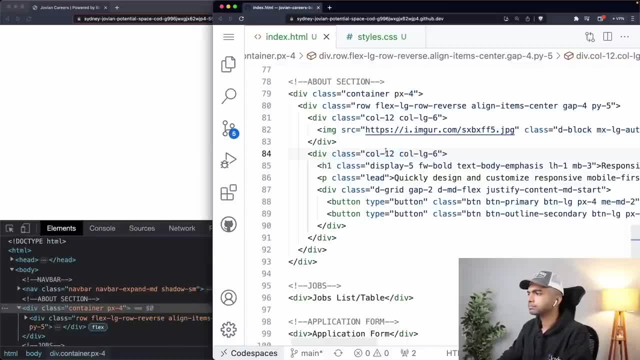 Okay, So let's give this call 12 as well, And on LG screens. Yeah, And on LG screens it's both of these are going to take up half width. Okay, So there seems to be this MXLG auto. I'm going to get rid of that. 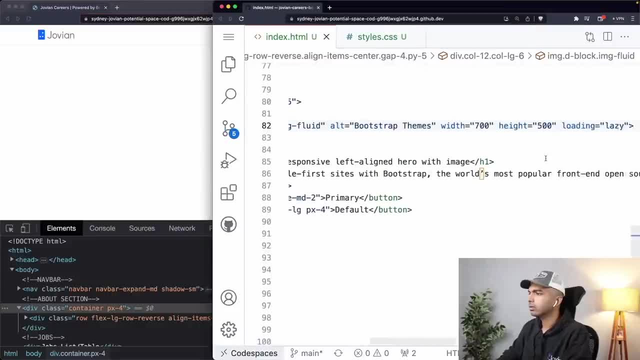 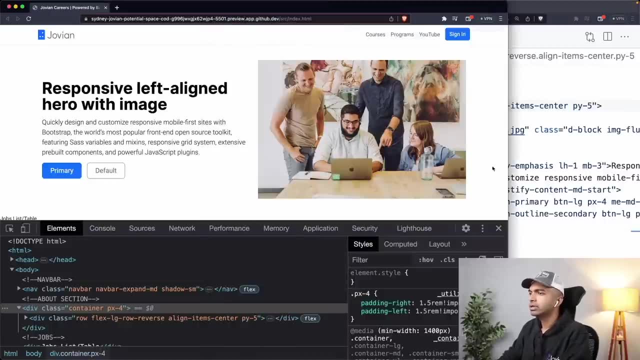 There seems to be this image: fluid. This is okay. What else? Well, I think this is a gap that might be causing the problem. We'll fix the gap later. Okay, So, yeah, So, till LG. it takes up the entire width. 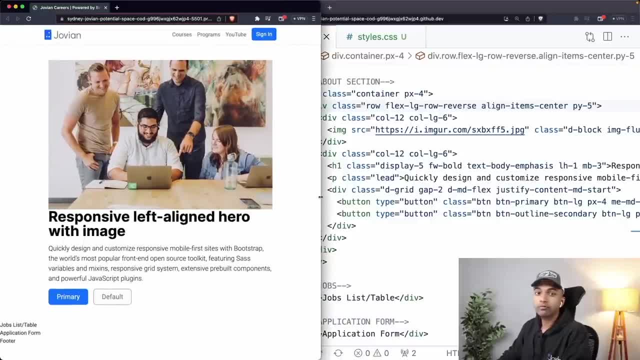 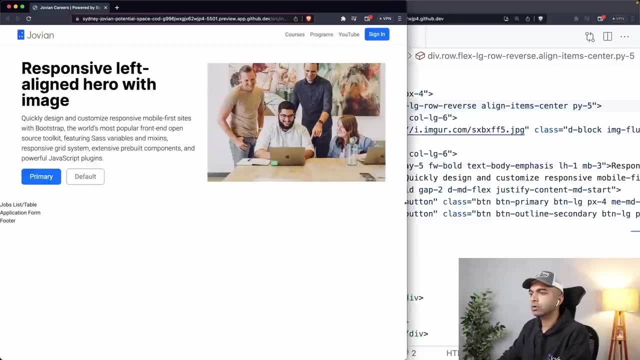 Okay, So, from the entire width of the width of the page or width of the container, the centered container, and from LG screens and bigger, it simply takes half the screen width. Okay So this is good. This is looking good so far. 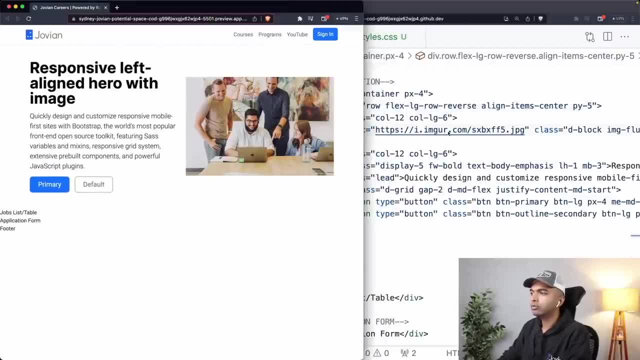 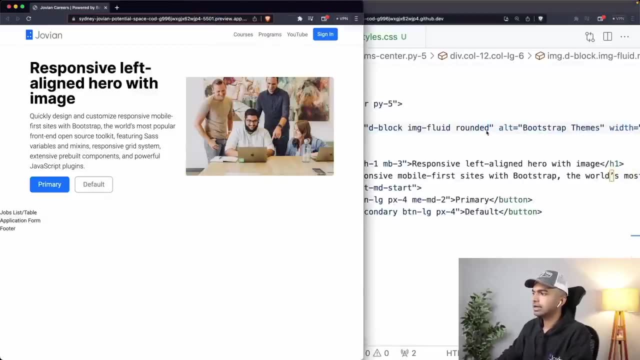 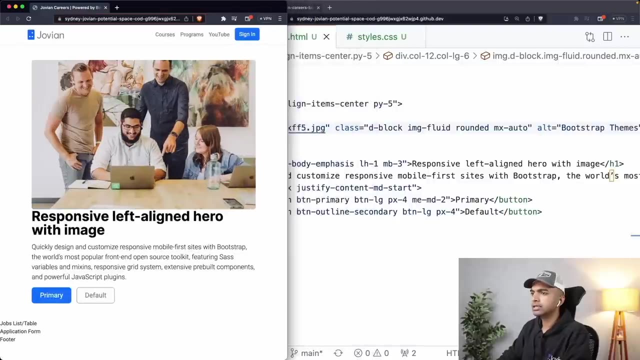 And let me also maybe add a rounded border to the image so I can just go in and say rounded. Okay. And let's also maybe say MX auto, so that it's centered on the page, no matter what width it's taking up, Okay. 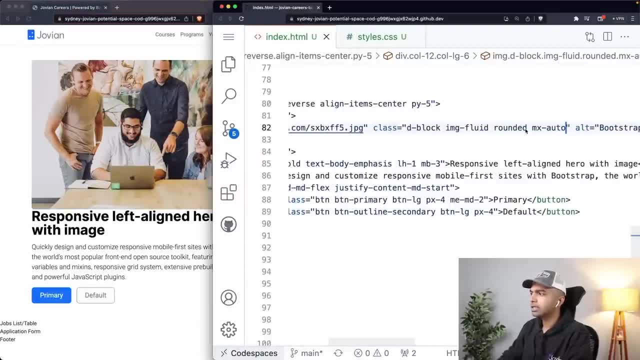 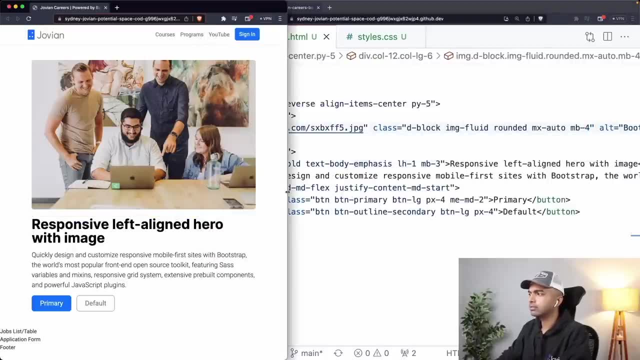 So let's maybe add some padding below the image. So let's just say MB or yeah, I think this is good. So now we've added some padding below the image and let's add a similar. we'll add a similar padding for the other content as well. 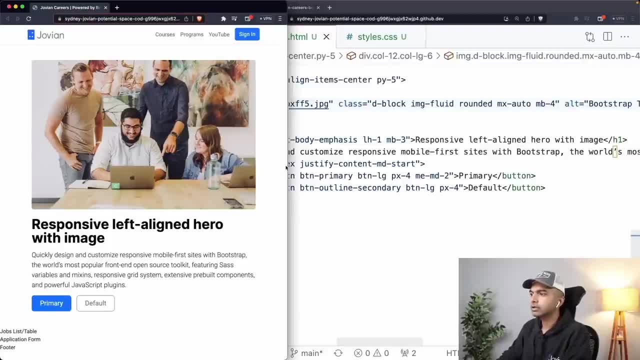 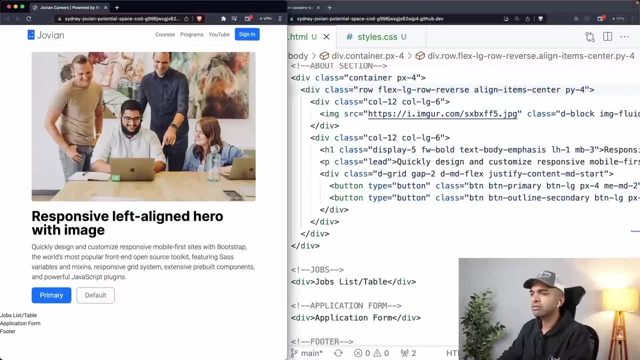 Okay, So this is looking pretty good. So now we have the Jovian logo and let's make this PY4.. I think PY4 should do the job for us, Yeah, So now we have the Jovian logo, We have this image. 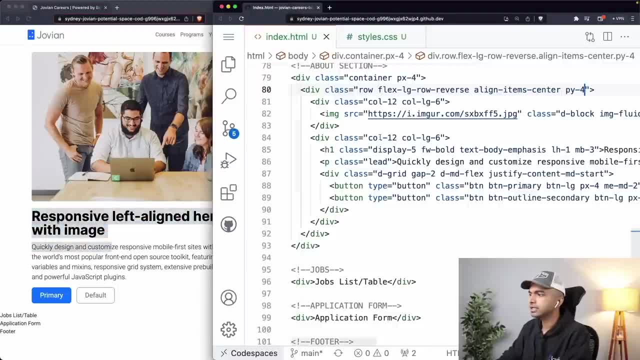 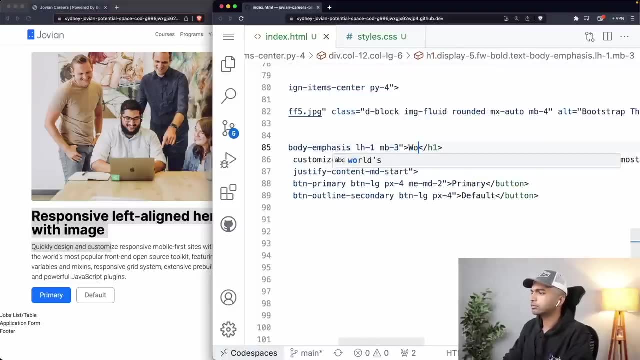 Okay, We have this text here. I'm going to change this text, So let's see display five: FW: bold text, body emphasis. All this looks good. I'll keep those LH1.. All that looks fine. I'm just going to change this to work at Jovian. 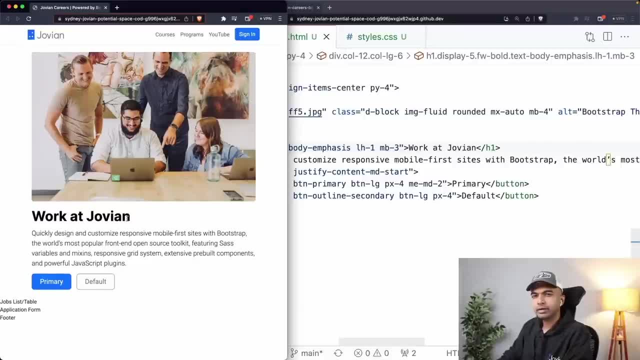 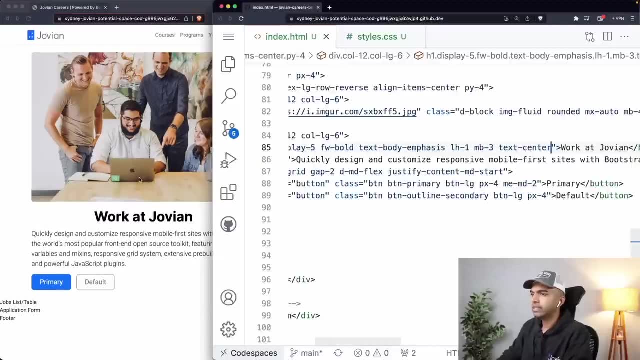 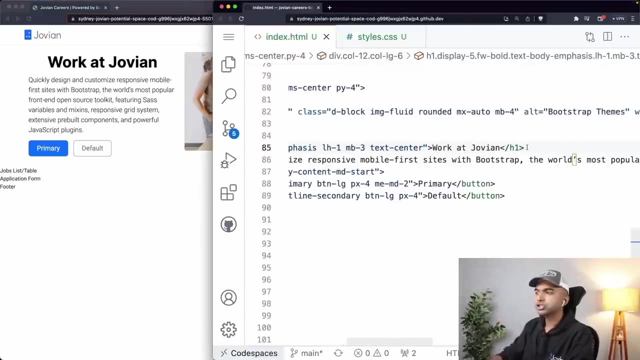 Okay, I think I want it to be centered by default. So I want to say text center by default, Okay, Then it's looking good. And then at a certain point I want it to become left align. So at LG, when the layout shifts, I want to say text LG left align to left align. 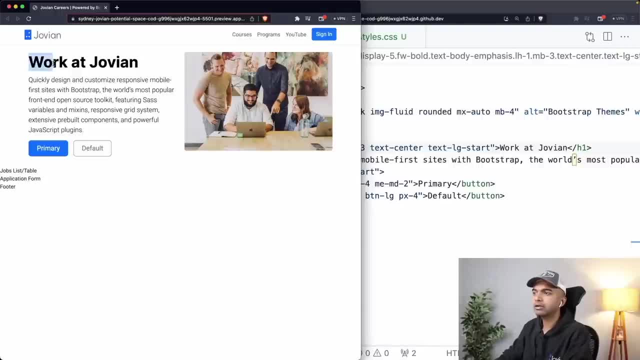 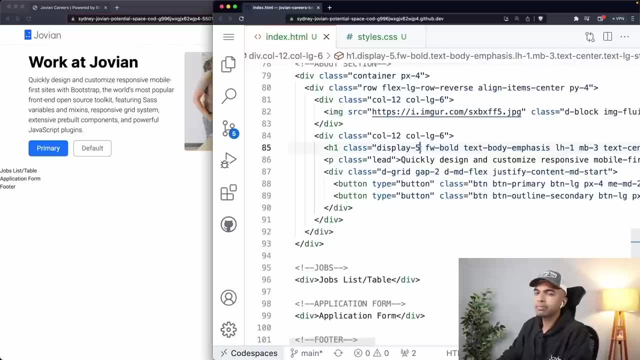 I have to say text LG start and it's going to become left align over here like that. Okay, Great, So again we've. you can try removing some of these and see what it does. What happens if you remove display five? what happens if you remove text body emphasis? 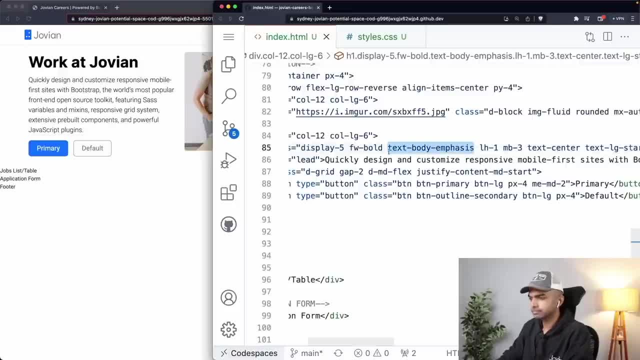 et cetera. Let's try it. Let's try it. Removing text body emphasis: Okay, It didn't make a difference, So probably we didn't need that. What about font weight bold? Do we need that? Okay? 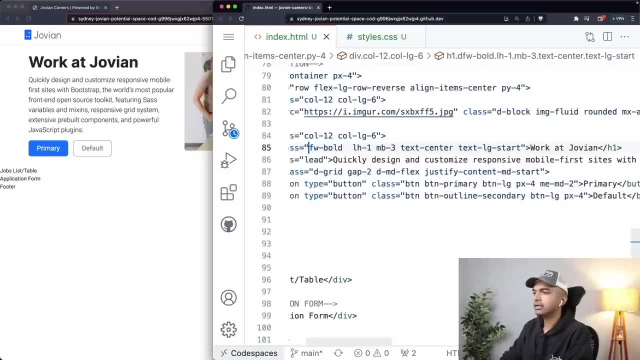 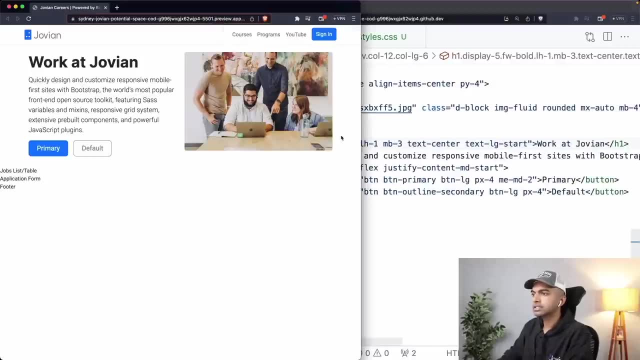 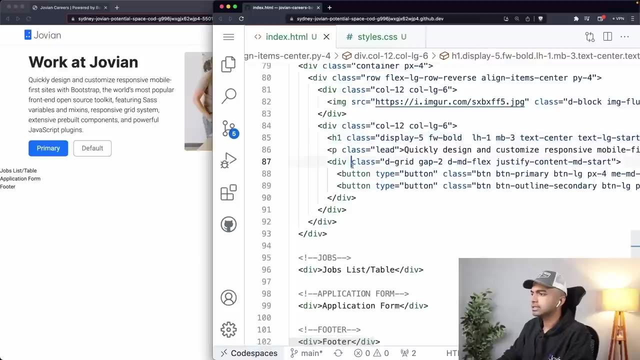 We definitely need that. What about display five? Do we need that? Yeah, we definitely need that. Okay, So this is all looking good. We have a work at Jovian. This is a nice little thing that we've added, and let's get rid of these buttons. 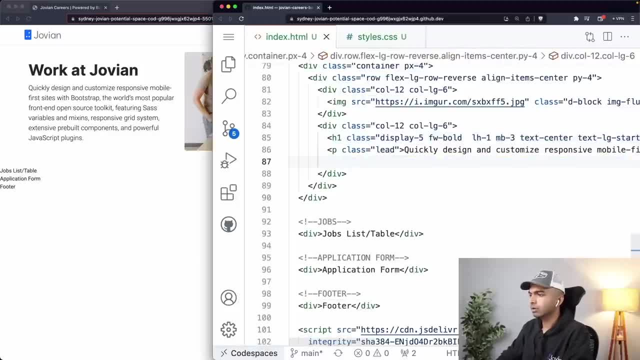 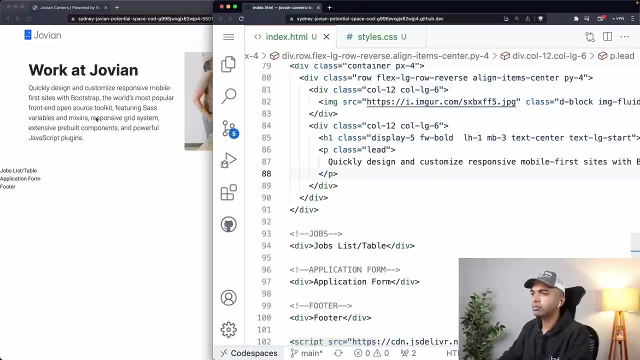 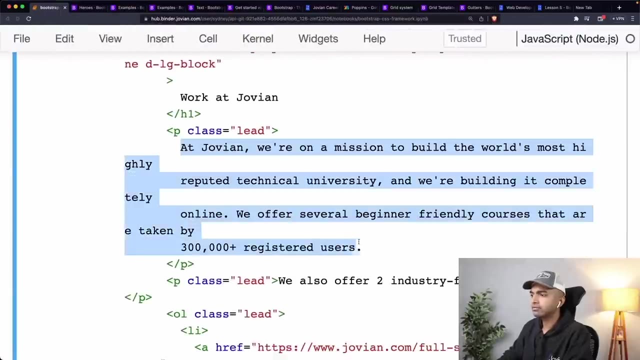 I don't need these buttons here, Okay. Okay, Let's take a look at this actual paragraph of text. I think this paragraph you want to maybe change it to the paragraph that we were actually using earlier. So I'm just going to come in and maybe copy over the paragraph that we had earlier. 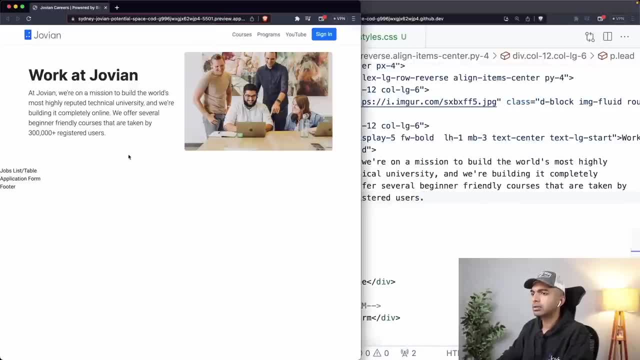 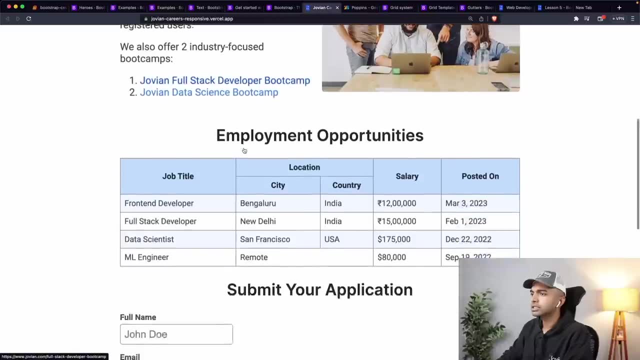 Let's paste this paragraph here. Okay, Looks good. Yeah, this is fine. I think we also had another paragraph linking to a couple of courses, So we had this full stack developer bootcamp, data science bootcamp- Okay, So let me add those paragraphs as well. 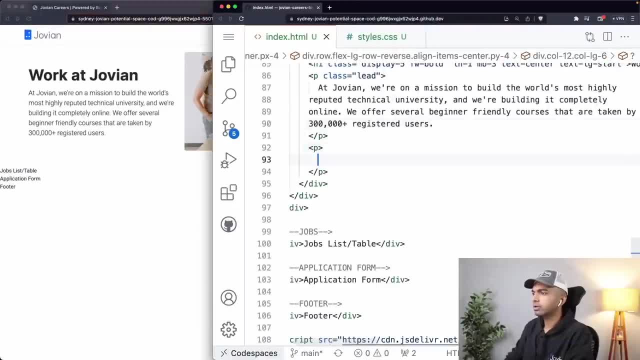 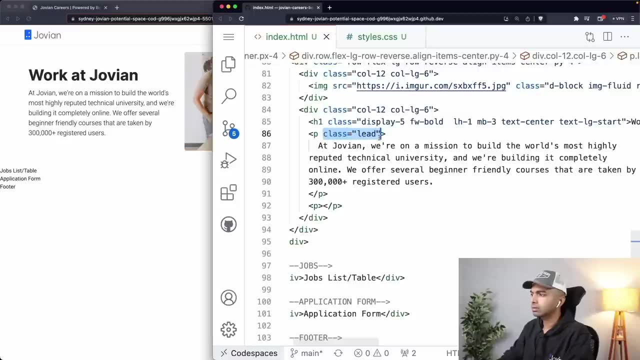 So let's add another paragraph and let's see if this class lead is important. What if I don't have this class lead? Okay, This class lead seems to be important. It's going to make the text a little nicer to read, a little bigger. 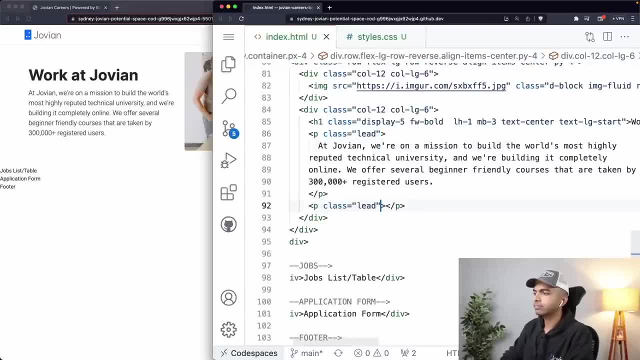 So I'm going to keep this, and I'm going to keep this in my next paragraph as well, And in my next paragraph, let's add this text: We also offer two industry focused bootcamps. All right, cool, And let's get the links to those bootcamps. 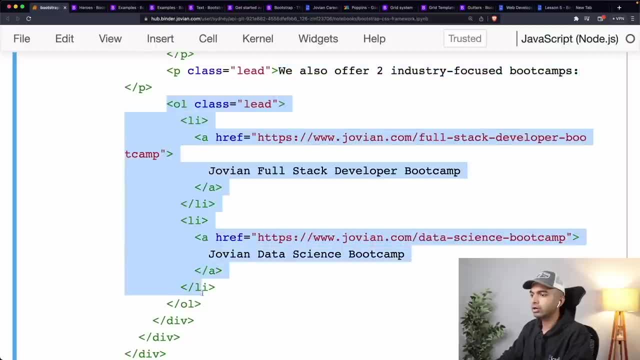 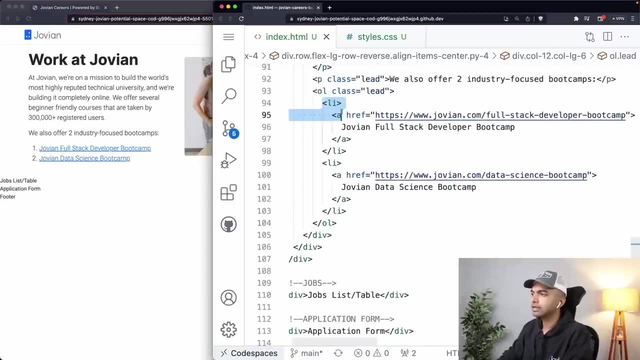 So let's get the. I'm just going to copy this entire ordered list. So we have an ordered list, Well, with the class lead. it contains one list item which contains a link to the full stack developer bootcamp. It contains another list item which contains a link to the data science bootcamp. 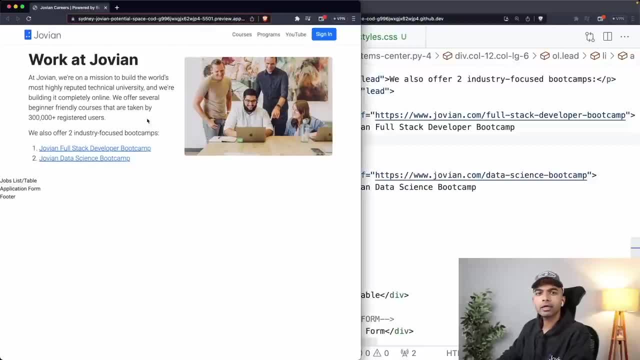 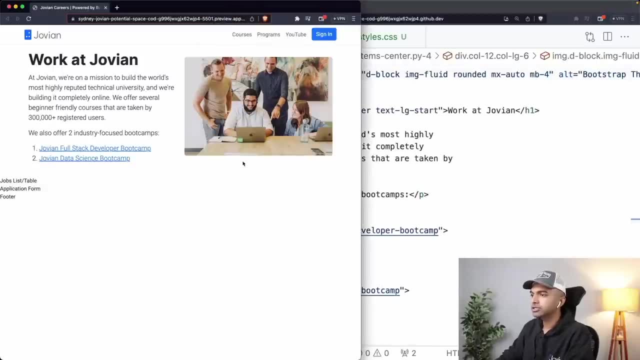 Okay, And just like that, we have created a very nice looking hero section, So this is often called the hero section. I think we can probably get rid of this margin. You can see that there's this margin bottom that we had kept. 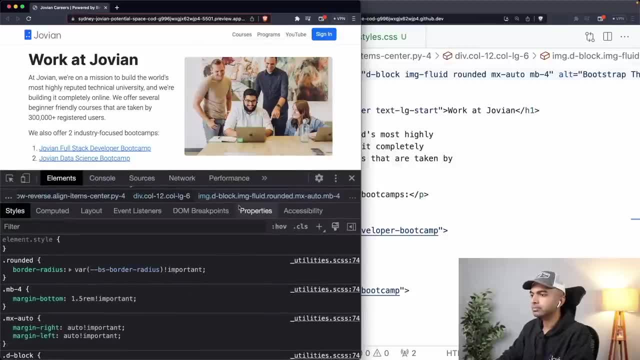 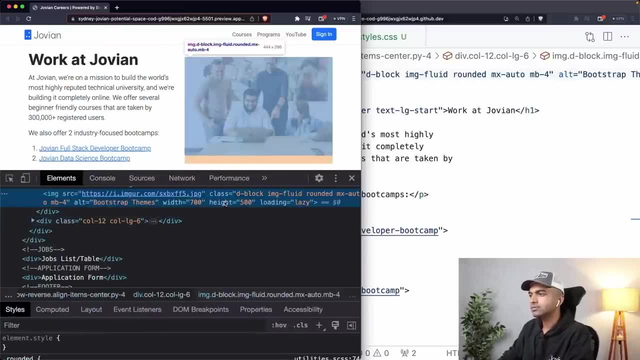 I think we can get rid of it when we get to a large layout. Yeah, So we have this margin bottom. I don't think it is very useful here in this case. So for the large layout, I'm going to get rid of it. 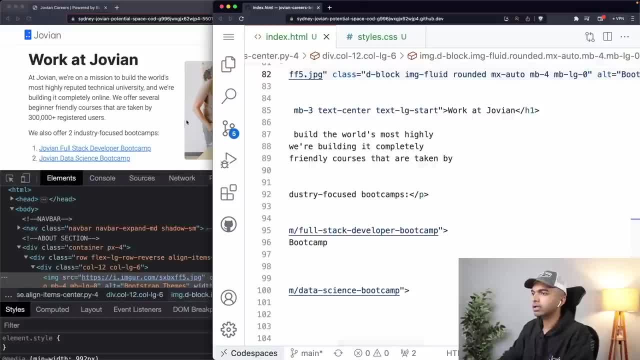 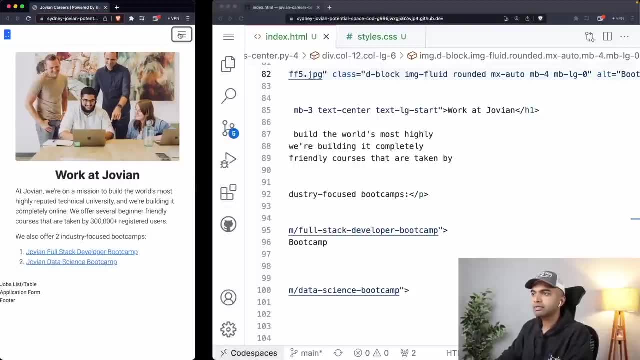 So I'm just going to say MBLG zero, Okay, nice. So now it's nicely centered on the page, Okay, Perfect. So on mobile screens we have this toggle and we have this image, We have the centered work at Jovian, but of course, this paragraph it's better to just 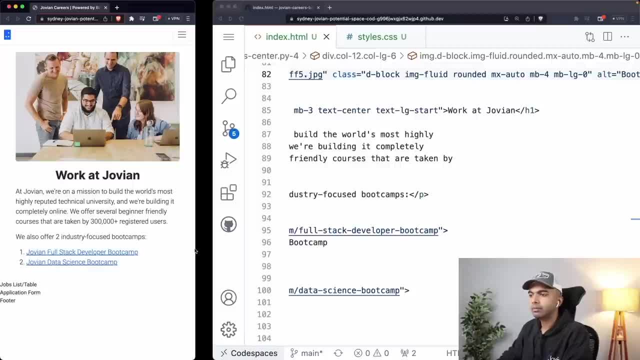 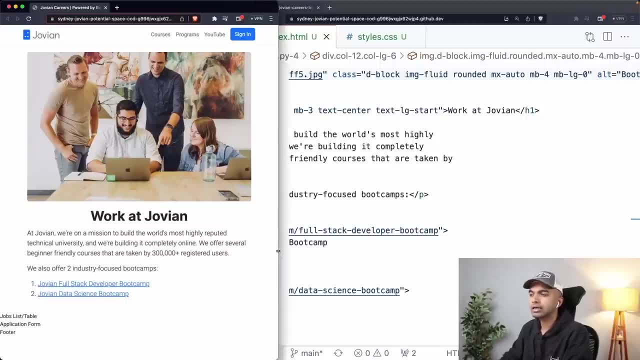 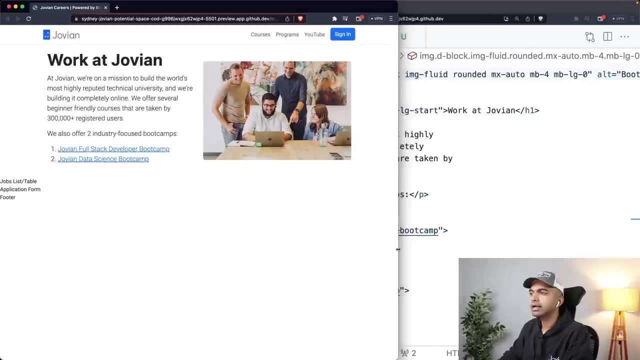 keep it left aligned. And then we have links, And then the font sizes are also responsive. You'll notice that the font size is actually increasing. That's what the display fonts or the utility classes allow us to do. Then, as soon as we hit this large layout, you can see that we flip into and then at. 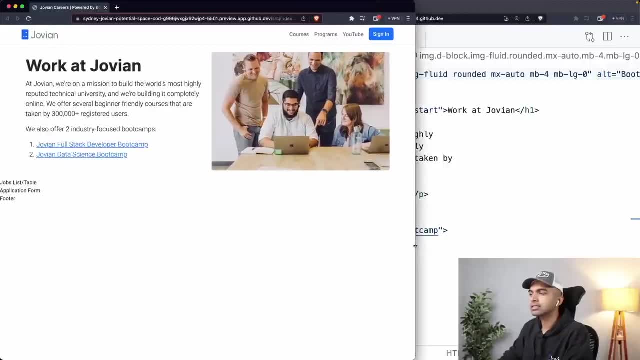 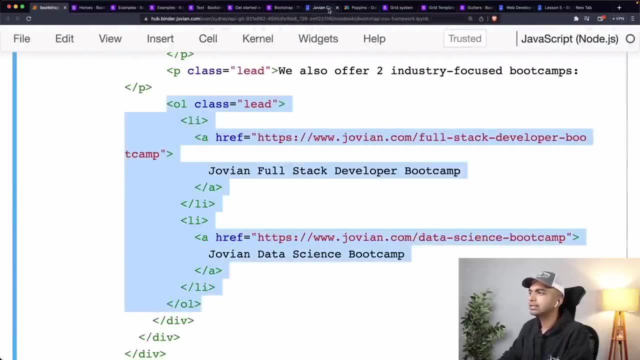 Excel. there's a certain change as well, Okay, In terms of the container size, but we flip into this nice two column layout, which is looking rather nice, And I don't think we need this banner image anymore, because just this layout itself is. 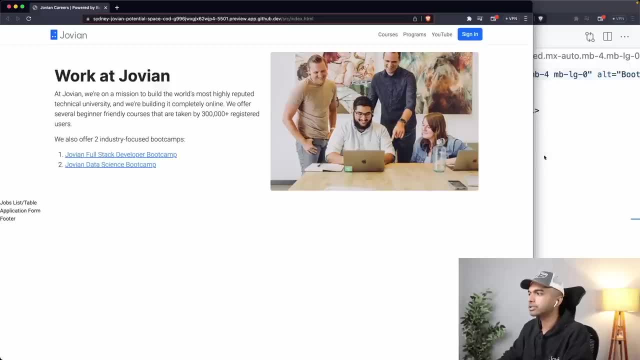 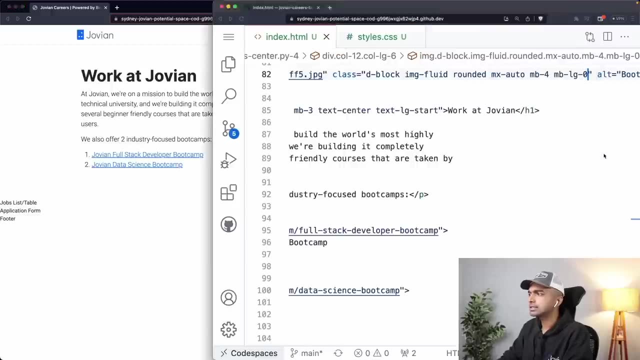 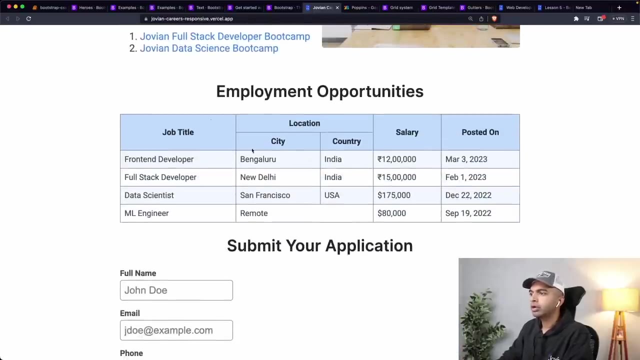 looking so nice that I don't feel like then further adding a banner image or anything. Okay, Yeah, Looks good. I am feeling pretty happy with this and now we can probably move on to the next section. Okay Okay, This is the employment opportunities which we want to show as a list of cards on mobile. 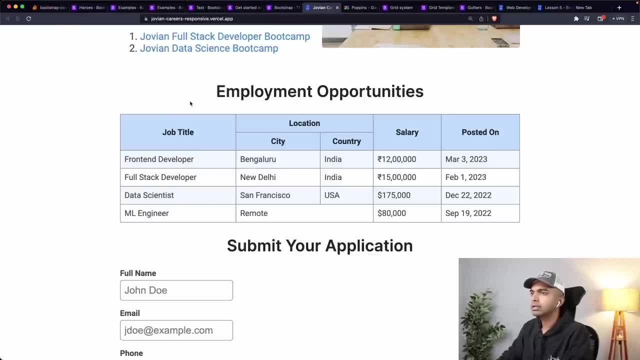 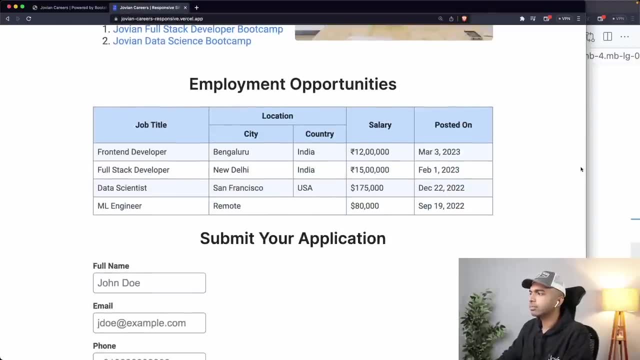 and on desktop We want to show it as a table. Okay, So how do we do that? Let me just copy this over here so that we can actually just see the side by side. So here you have this employment opportunities table. by default, it's a list of cards like: 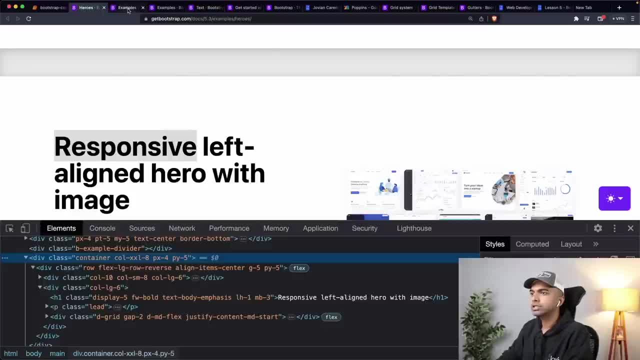 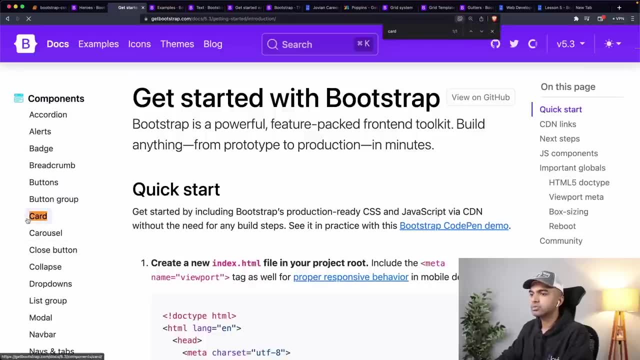 this. Let's see if there is something to create cards in bootstrap. Let's go into the bootstrap documentation. Let us search for cards, Okay, Cards, Yeah. So there seems to be this card component, and this card component can be used to show an. 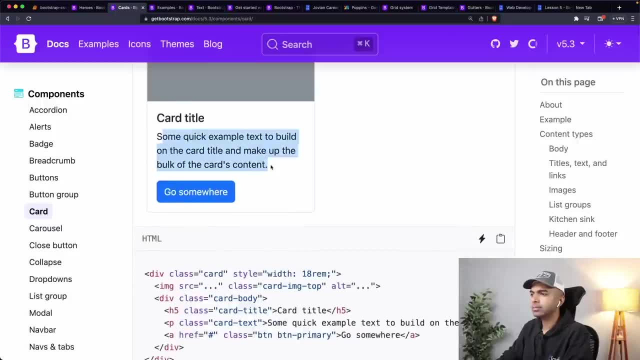 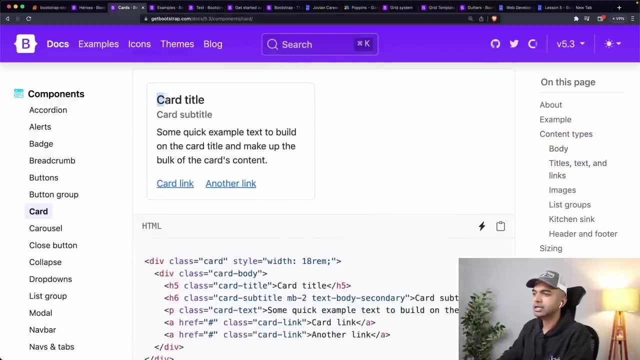 image can be used to show a card title, used to have have some texts and maybe also have some content here at the bottom. I need something much simpler. Maybe I need something like this, which has a card title or subtitle and maybe just some. 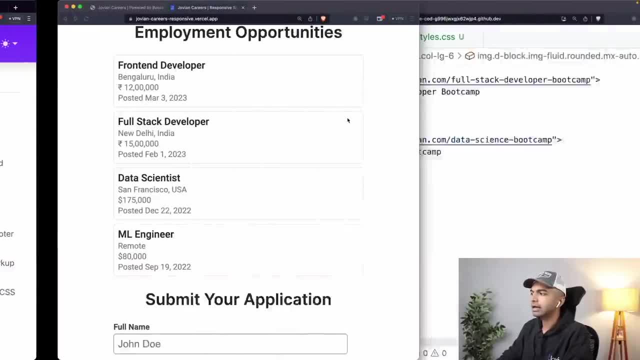 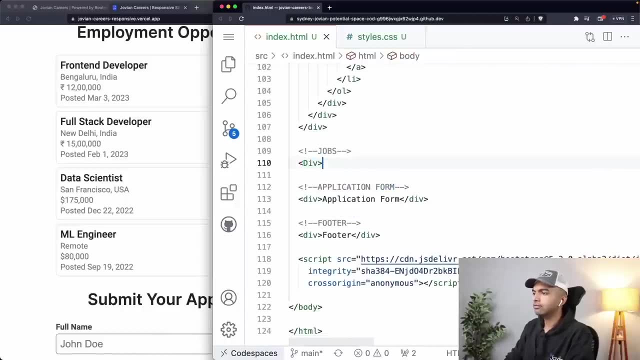 text about it. So I'm just going to copy this and I am going to come in here. I'm going to create a new section Again. I'm going to create a div And I'm going to give it the same class that I had for the previous div above. 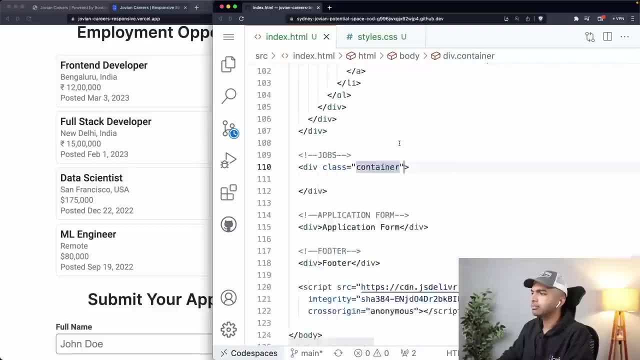 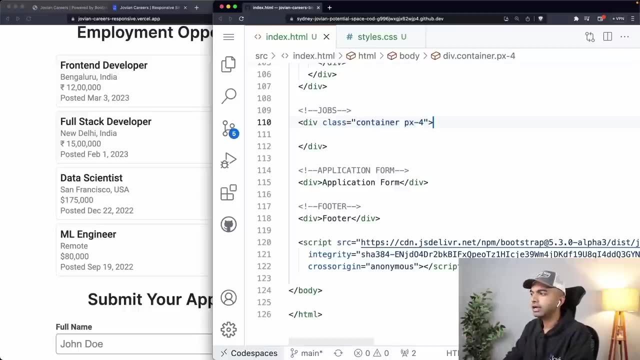 So container, let's see what did that look like? container and PX four. So I'm going to give it container and PX four, So that left and right we have some space, so that the content does not stick to the left end of the page. 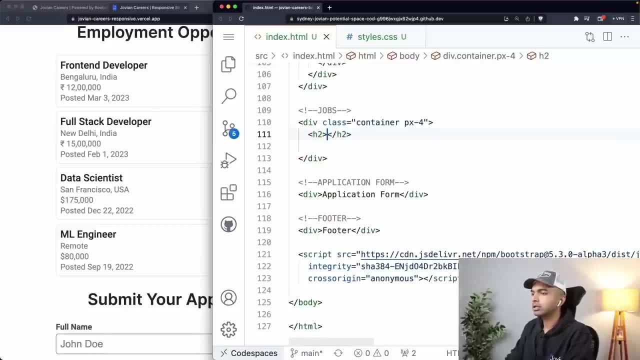 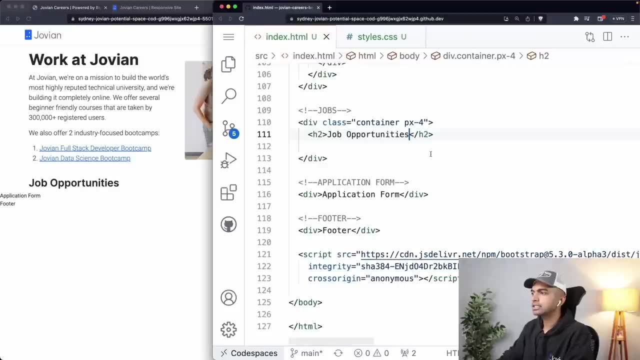 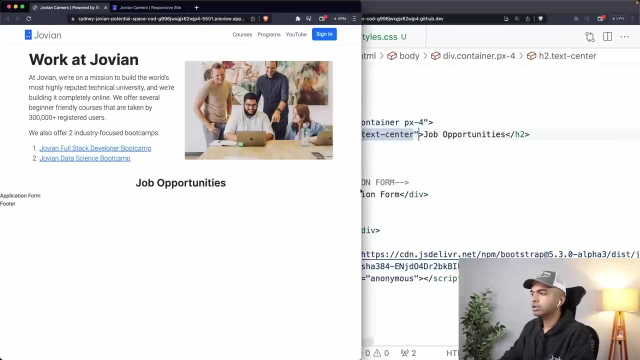 And let me put in an H2 here and let me just put: let me just call this job opportunities, Okay. So now we have this job opportunities, Okay. So let me just add class text center here, Okay, And I want to right now, I want to just work with smaller layouts. 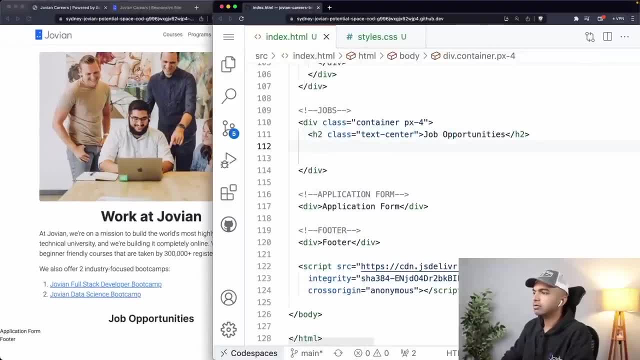 So I'm just going to keep it like that. And let me just now add this: Maybe I'm going to add a div and I'm going to give it the ID: jobs list. Well, maybe I don't really need an ID. Let me just drop in a comment here saying jobs list. 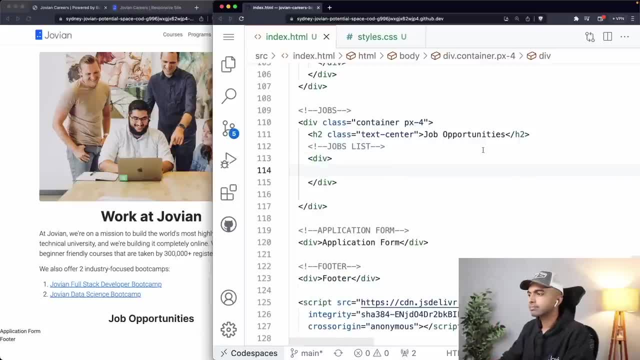 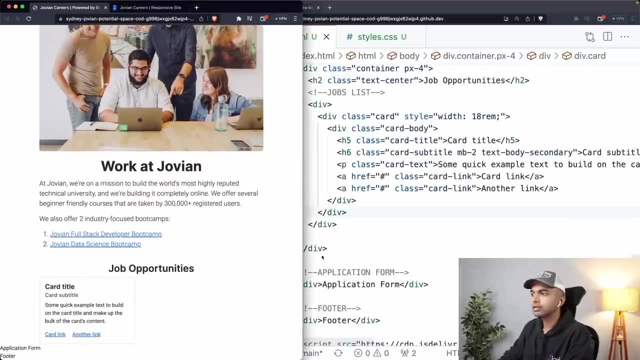 Okay, So inside this div is where I'm going to create my cards, All right, So let me paste in this card and let's see what it gives me. Okay, So this is the card that I get. it's on the left. 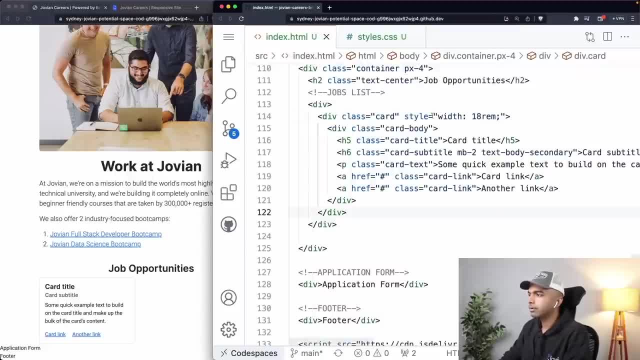 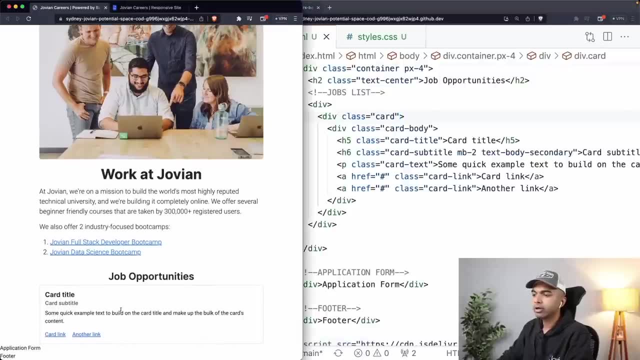 So I'm going to change a few things up. first, I'm going to remove this with. I don't need this with. I don't need this class card, because that's what adds this nice border around it. I am going to add maybe a M Y four, which is just okay. 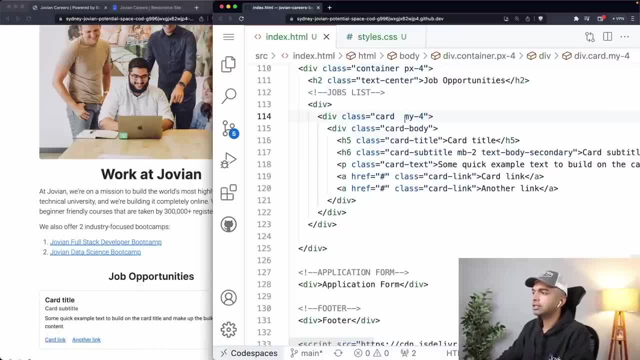 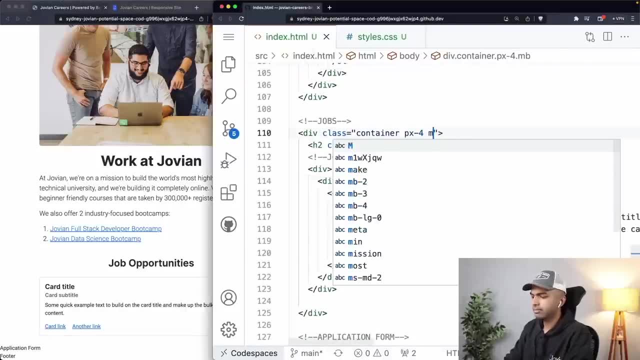 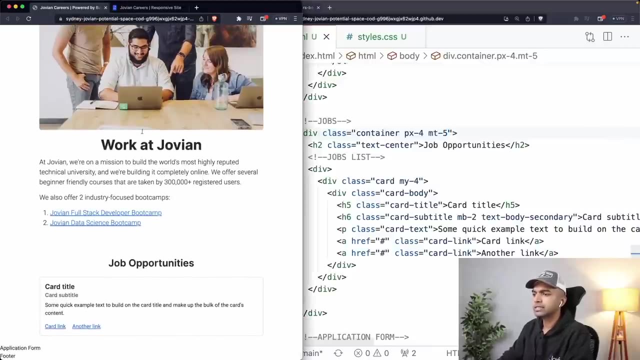 Maybe not here, Yeah, So which is margin in the Y direction, four units, which is going to just give us some space here, And maybe I'm going to also add a M E five here, Yeah, So that this is a little spaced out from the previous content. 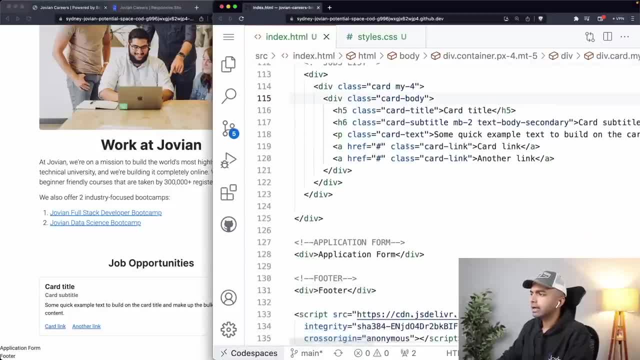 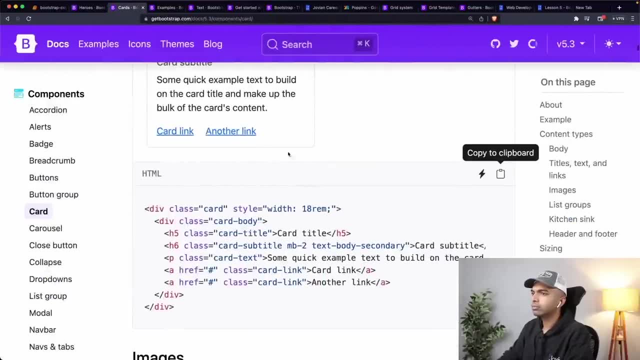 Okay, Looks good so far And let us now add: okay, let's now fix the card title, So we have this front end developer role. Okay, So let's grab the content of the front end developer role here. Okay, So card title is front end developer. 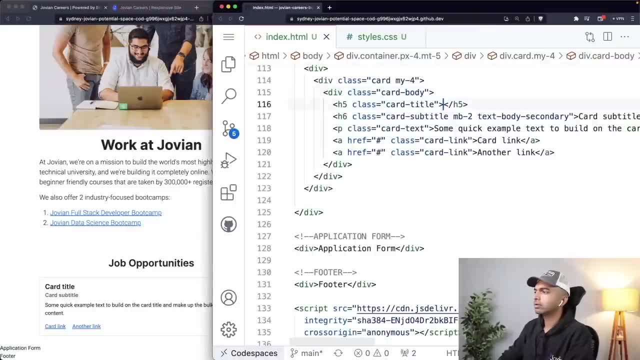 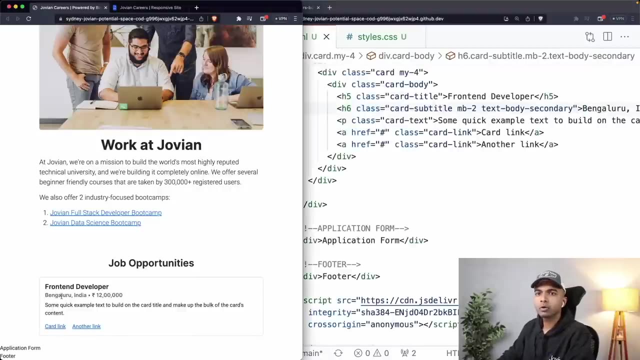 So I'm just going to use that Front end developer. Okay, That looks fine. Then we have a subtitle. in the subtitle I'm going to put in the location of the job, which is Bengaluru, India, and 12 lakh rupees, which is the annual salary. 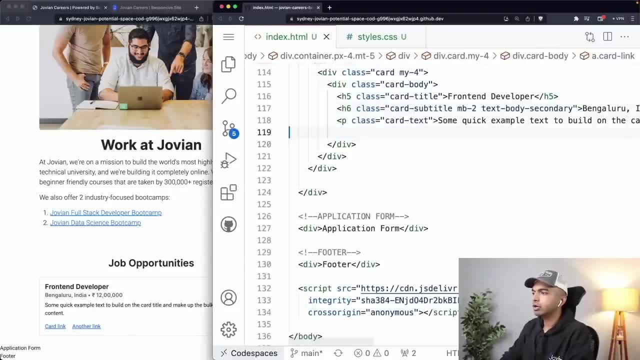 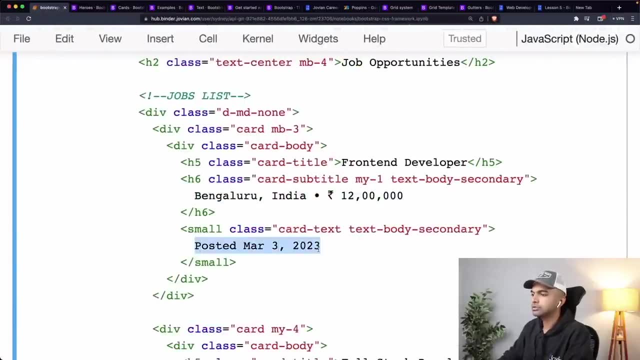 So I'm going to put that in here. I don't need these links at the bottom, So I've gotten rid of these links. And then I here. maybe I can just put in that this was posted three. This was posted like on March 3rd 2023 or something like that. 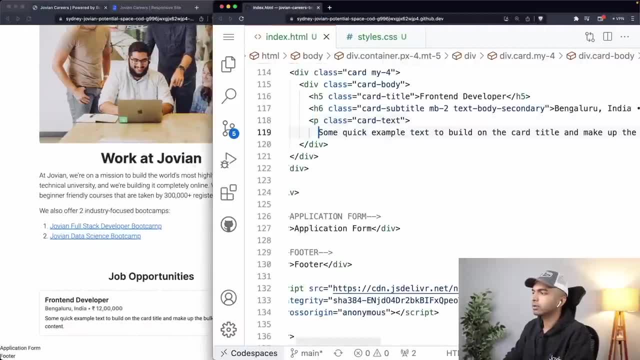 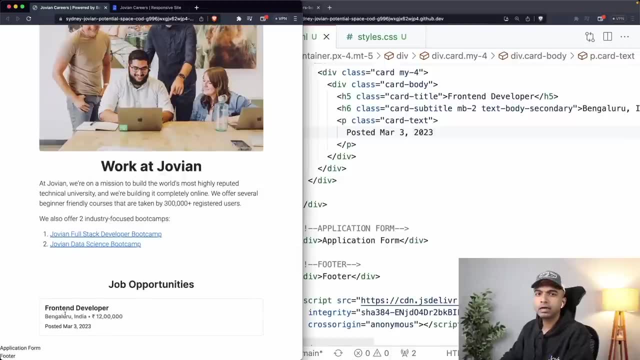 So I'm going to put in that information over here. Okay, So very basic content. Yup, Okay, So now I have front end developer. This is good. Bengaluru, India, March 3rd 2023, looking good. 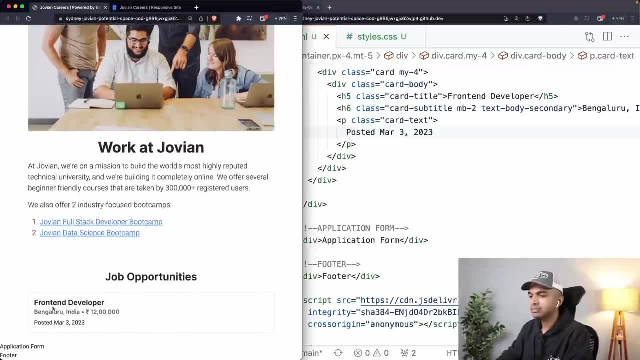 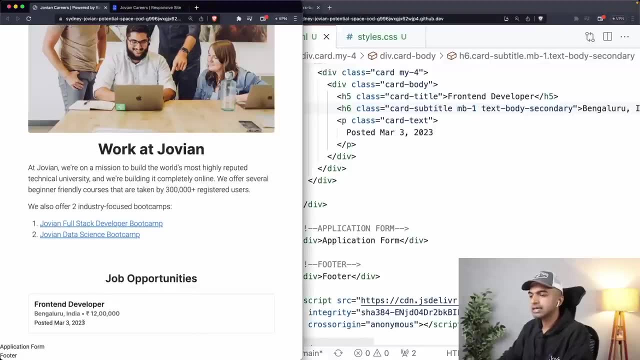 I can maybe just make this slightly better. Okay, I think the spacing is a little off, So maybe this MB2 is not required. Maybe just make it MB1.. This looks fine And I guess this text can be slightly smaller and maybe a little grayed out. 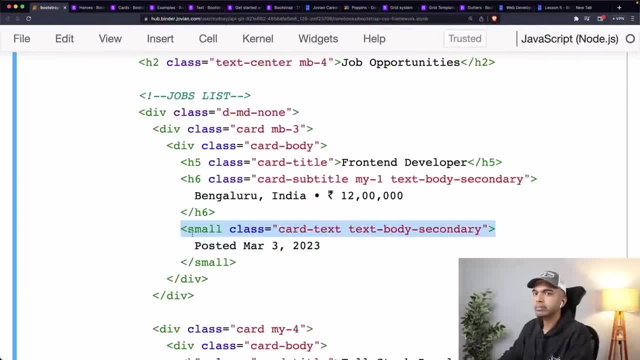 And that is where I can use this small tag, HTML tag, which bootstrap automatically turns into slightly smaller text, And I'm also going to use text body secondary. So I still have this card text class, but instead of using the P tag, I'm using the. 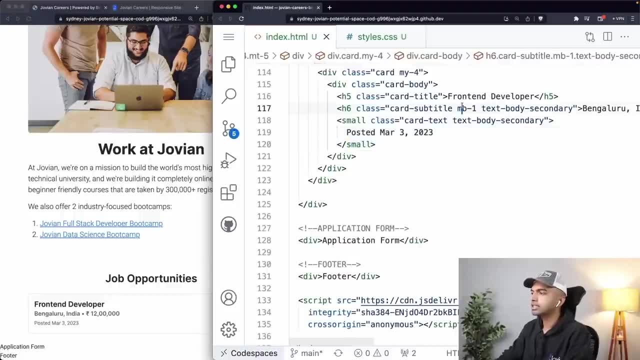 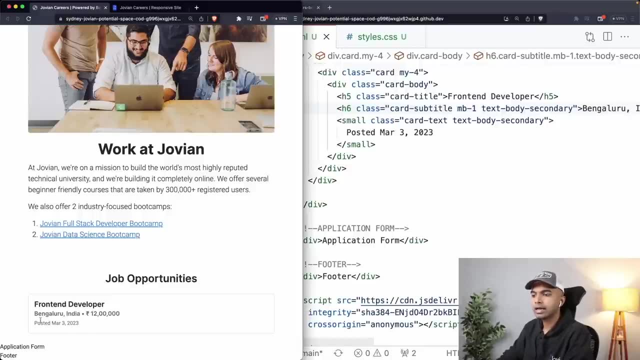 small tag and I'm using the color text body secondary. So now you can see that we have this nice hierarchical card where we have this front end developer: Bengaluru, India, 12 lakh rupees and posted March 3rd 2023. 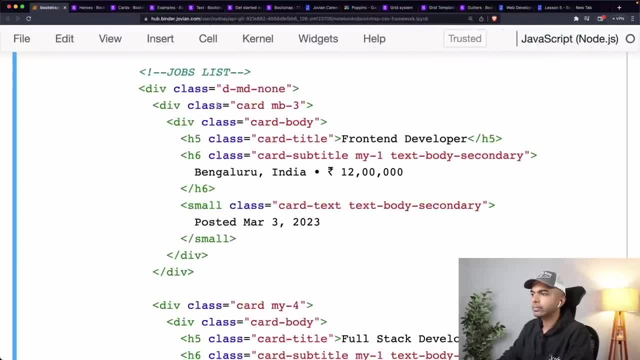 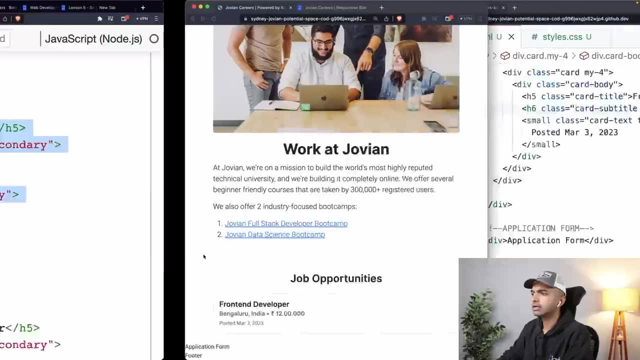 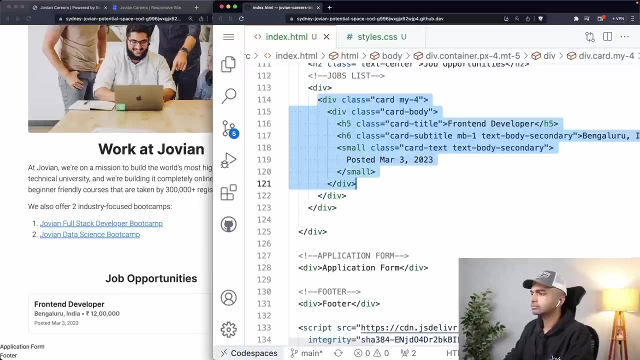 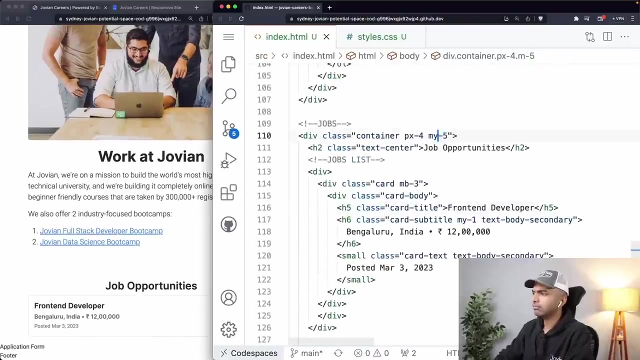 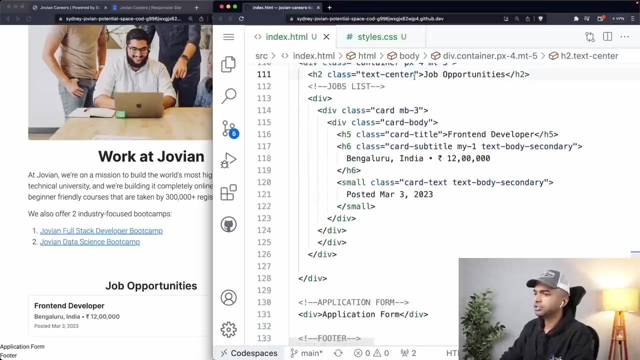 Okay, So that is the yeah, so that is the card that we have created, And I'm just going to copy this over just so that we have like a nicer version of this available for us to easily replicate. Yeah, And let's fix this padding here as well. to my five: empty maybe this edge to need some. 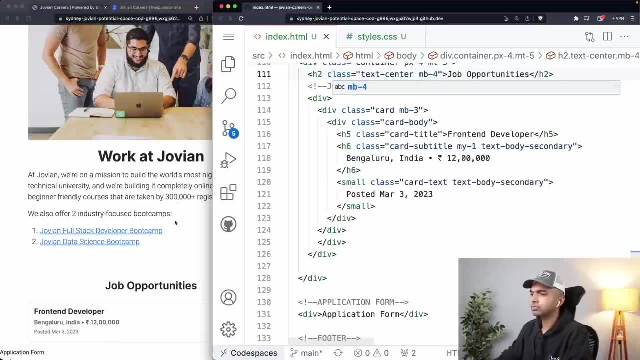 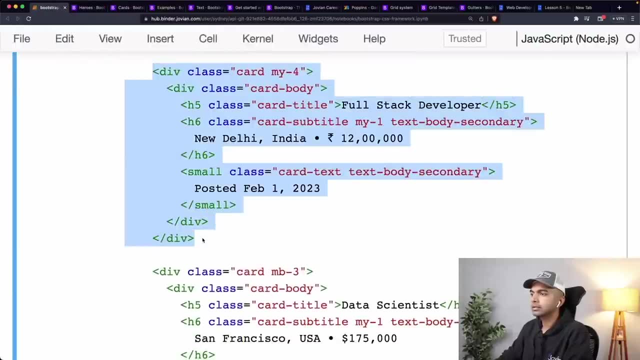 padding below. So I'm just going to add MB4 to this edge too. Yeah, So that things are a little spaced out. Okay, So that's one card. Let me copy over the other cards as well. So this is the full stack developer role. 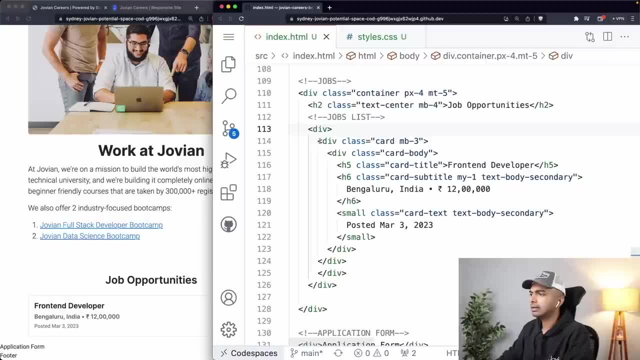 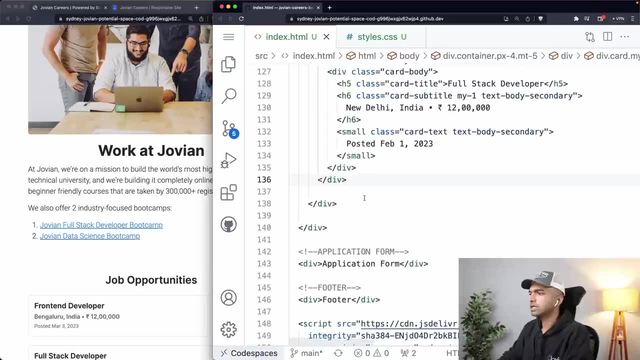 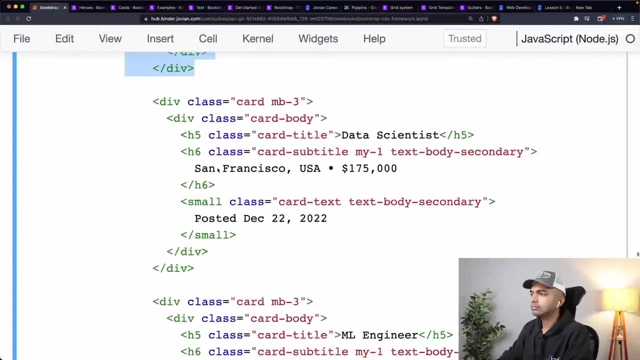 So let me come in and let's not Okay. Okay, Now it looks like I have this additional dev here. full stack developer role. Let me just format the document Looks fine, Okay. Full stack developer. Let me add in the data scientist role as well. 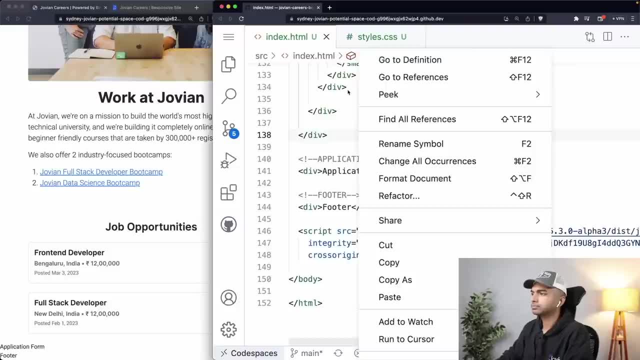 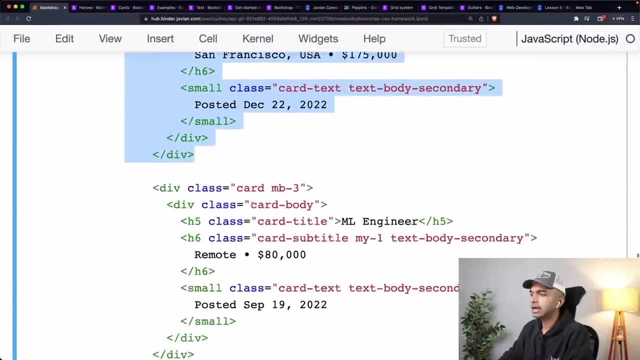 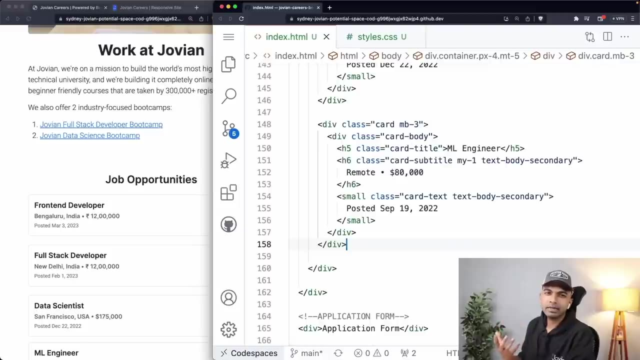 Data scientist. that is the data scientist role right here, And finally, let me add in the ML engineer role as well. Okay, So what we're doing is simply using the classes from bootstrap. We're still using writing, plain HTML code, but now we're adding classes from bootstrap. 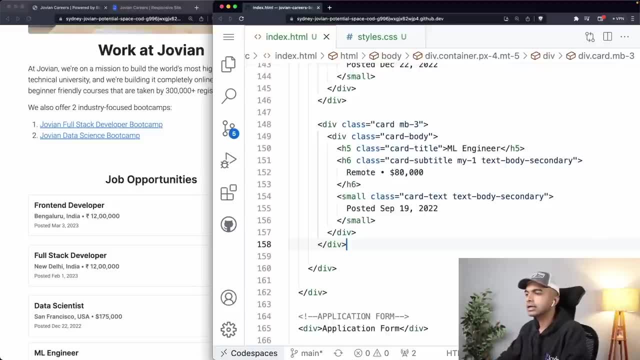 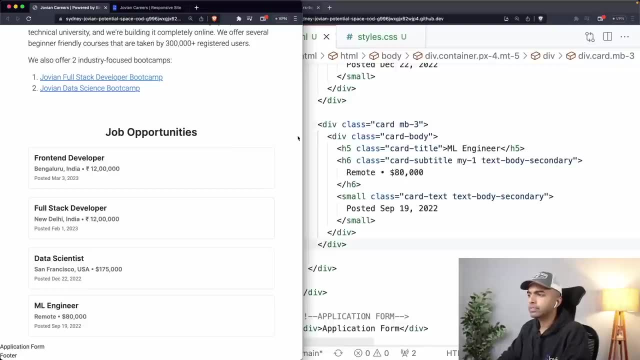 and all those styles and maybe also some JavaScript. nice features can get added in automatically via bootstrap. So now we have all of these job opportunities. I think this is looking pretty good. This is fine, but I don't want this to show up beyond MD. 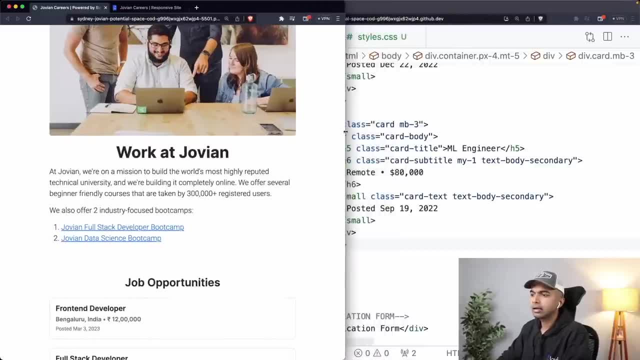 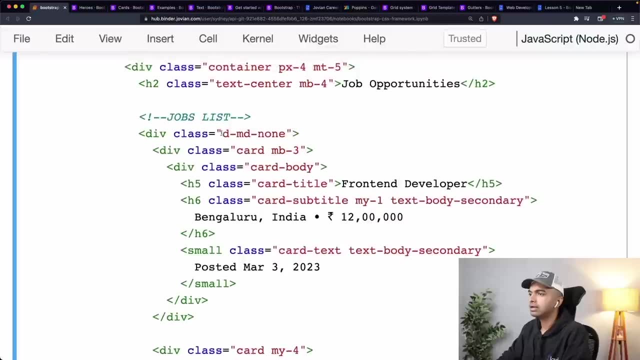 So I think when we hit the MD breakpoint, I wanted to, I want this to disappear. So that's where we have- Okay, We have this DMD none class, So we can say that by default it has a certain display, but at the MD breakpoint, we want. 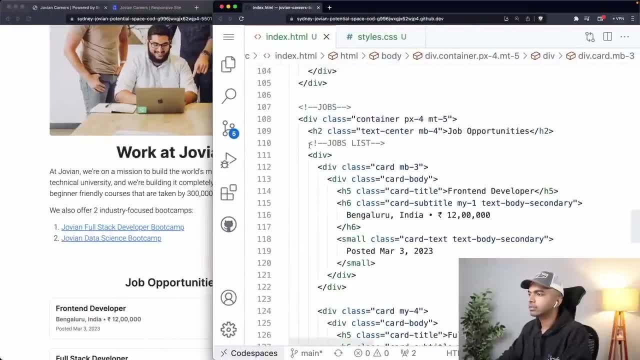 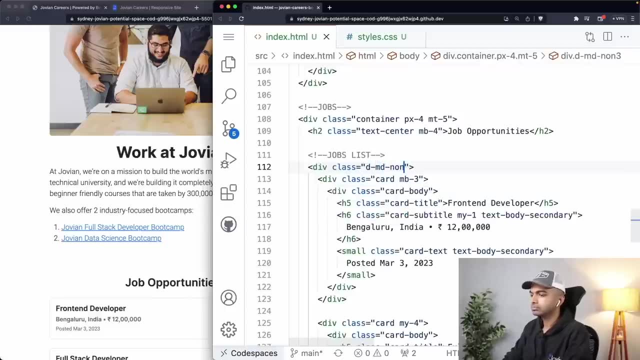 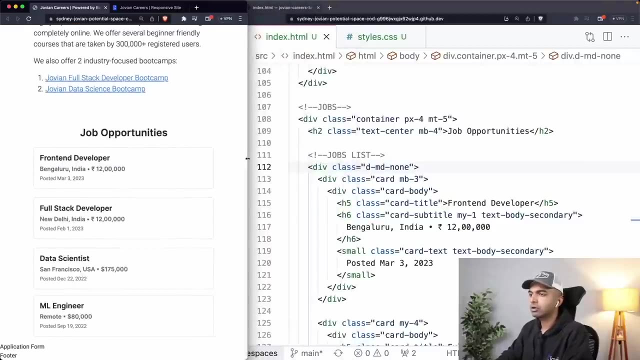 it to disappear. So for the entire jobs list. but this is the jobs list. I'm just going to give it the class D MD, none, Okay, So you can see that that's in very small screens. This is visible and this is looking good. 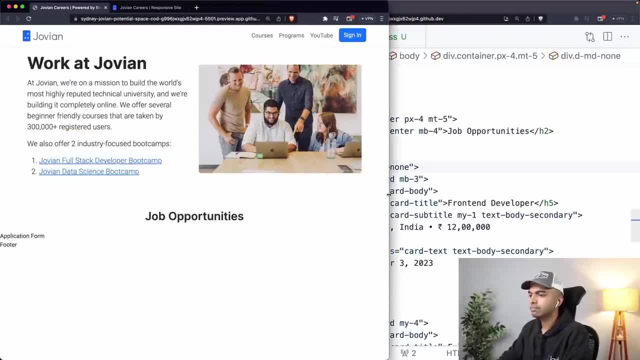 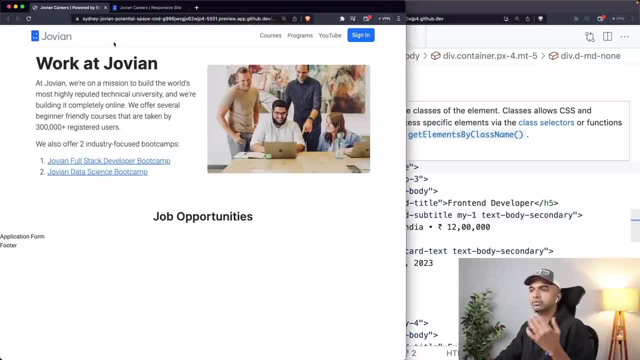 As soon as we hit the MD breakpoint, Then this goes away and is no longer visible. Okay, So with that I think we've completed the first one, or the first half of the page, which is the nav bar, the hero section and the job opportunities, at least on the mobile view. 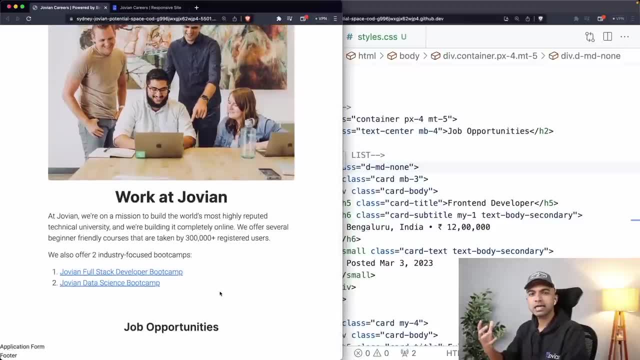 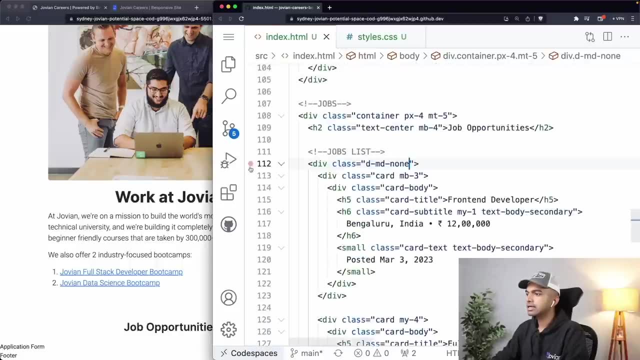 Now, of course, at MD this disappears and from size MD. we want to show a table, So let's maybe first bring in a table here. So inside the jobs list, well, right after the jobs list, but still within the jobs. 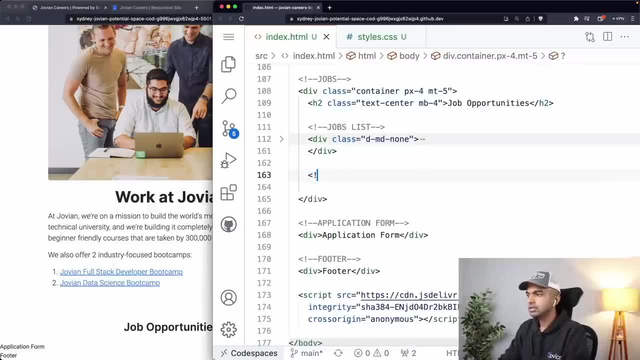 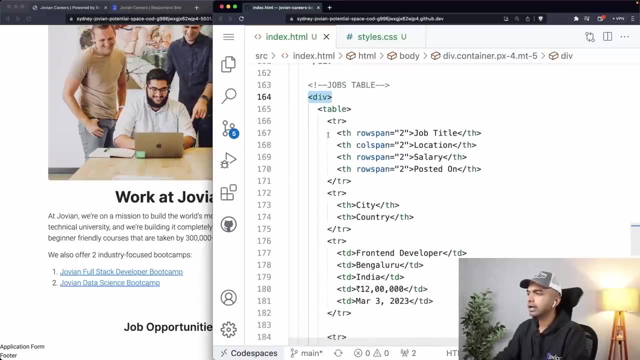 Dave, So within the jobs container we want to add a table. So let's just add a jobs table here. Okay, And let's first- maybe I'm just going to put in a div containing a table. So you can see all I've done here is I've have a div and inside the div I have a table. 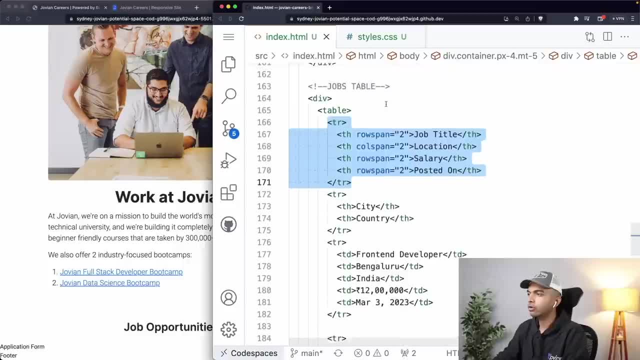 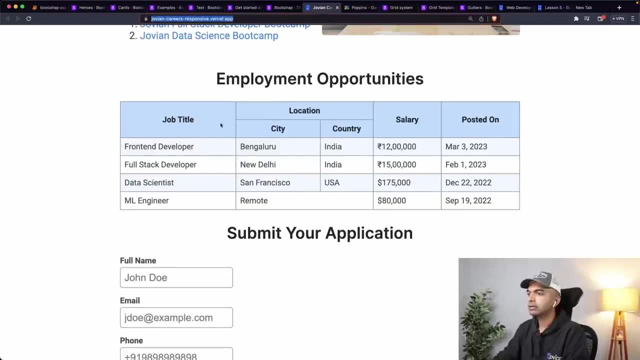 and inside the table I have this table row or the header row, And of course I've used certain call column spans and row spans to achieve this kind of layout where you have no job title, then location has city and country under it, and so on. 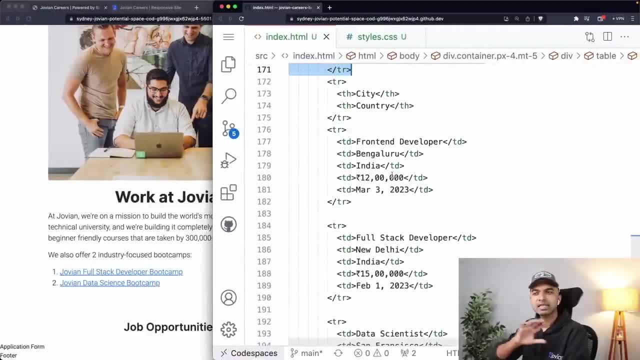 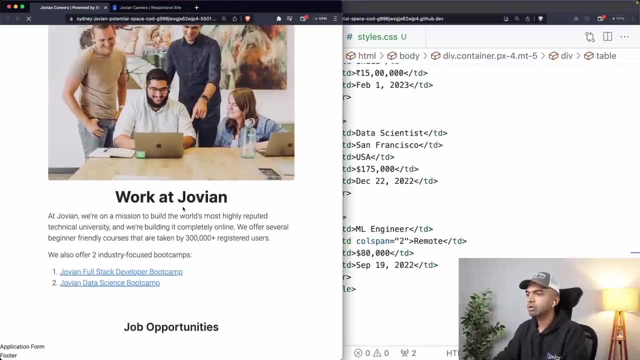 But to achieve this layout, I have used column span, row span. So this is the exact same table in terms of the basic HTML that we had the last time, And I'm just going to save that and let's see what that does. So now this is added, this table here at the bottom right. 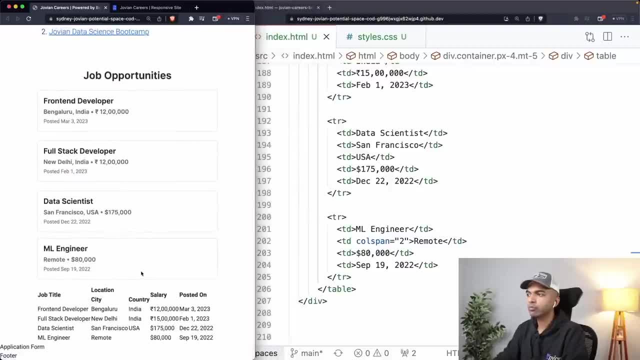 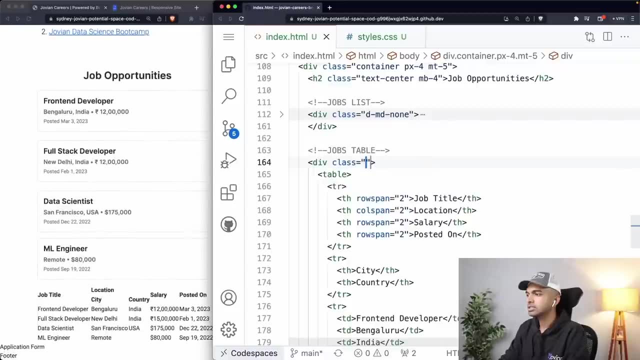 But there are two issues here. One is that this table is always visible. We don't want it to be always visible. We want it to be visible only on MDM Okay And higher. So I'm just going to say class D, none. 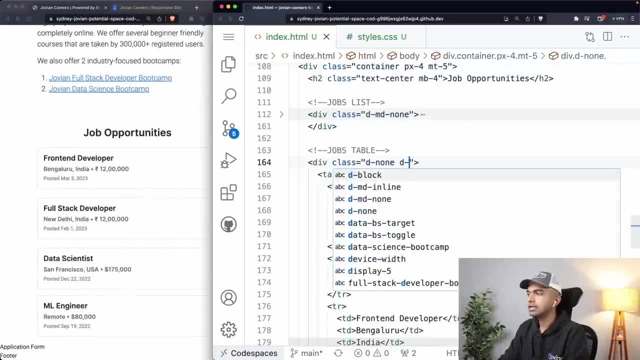 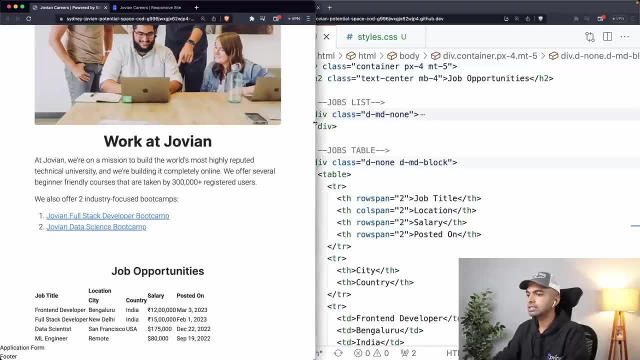 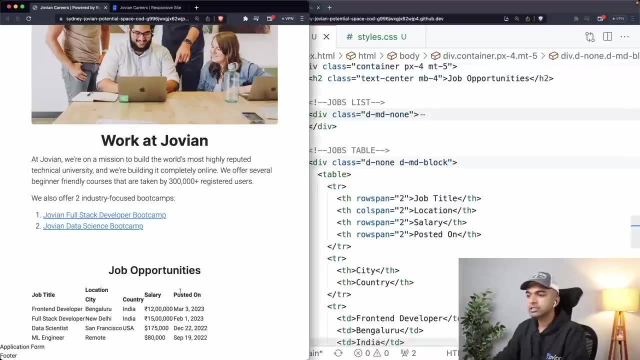 So, which is by default, we don't want it to be visible. and then DMD block, Okay, And what that does is: from MD on MD, the list disappears and the table appears. Okay, That's good. The second thing is, of course, this table is not looking very nice right now. 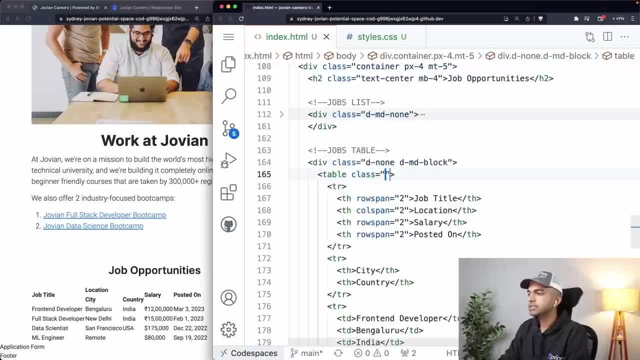 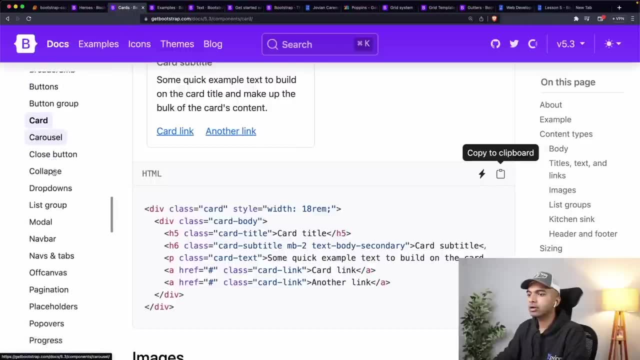 So one thing we can do to trigger bootstraps tables Is simply use the table class. And how did I get this? Well, I simply looked up the documentation. So in the documentation, just search for table and they have this class for table. 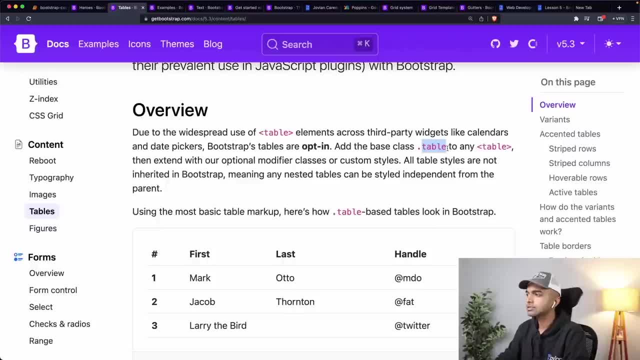 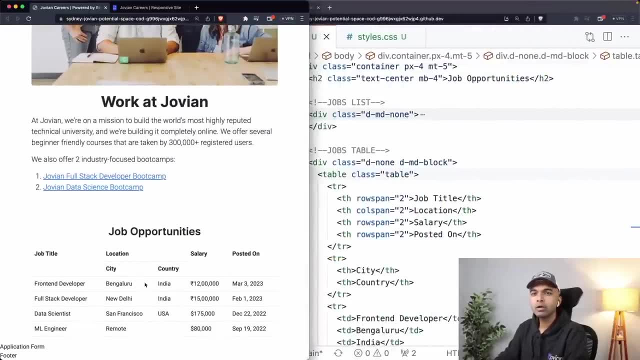 So you can just add in table the table class to any table component and that's going to create this nice table for us. Okay, The table is looking nice, but we still want borders around the table, So you want a border table. 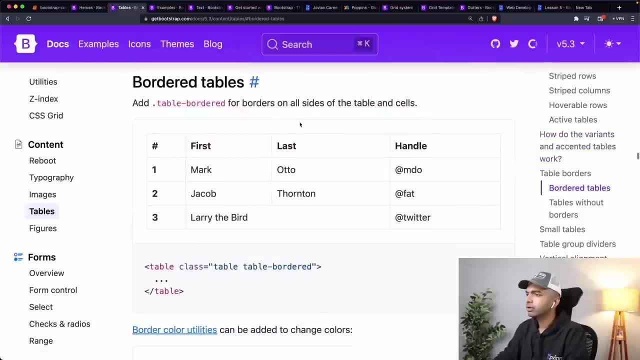 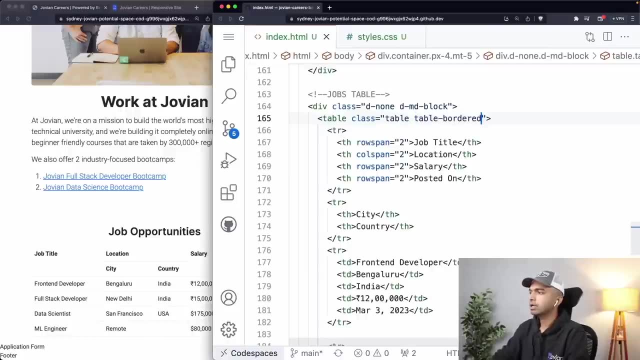 So let's see where. how do we add a border to the table? Well, it looks like we just have to add the table bordered class. So I'm just going to come in here and I'm going to add the class table bordered. 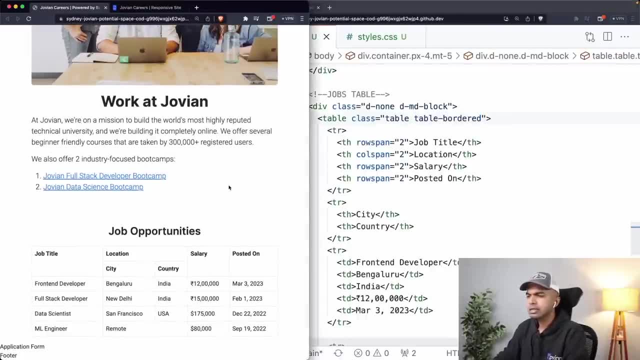 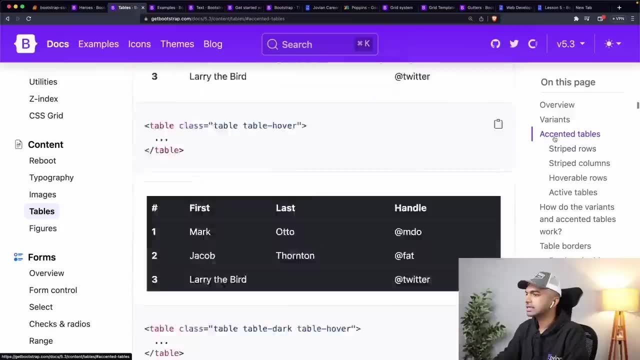 And voila, our table now has borders- Pretty good. I would like to maybe give it some more color. So let's see how we can add colors. So, accented tables: well, let's see how we can maybe make get these striped rows. 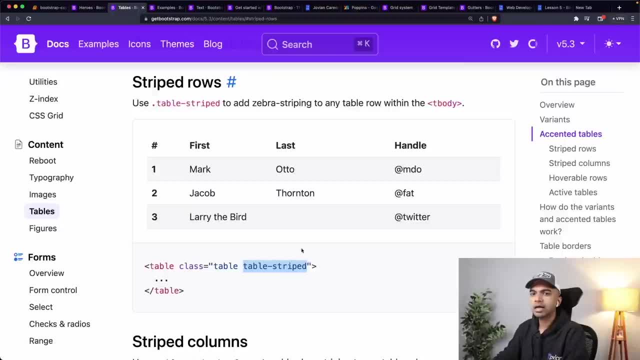 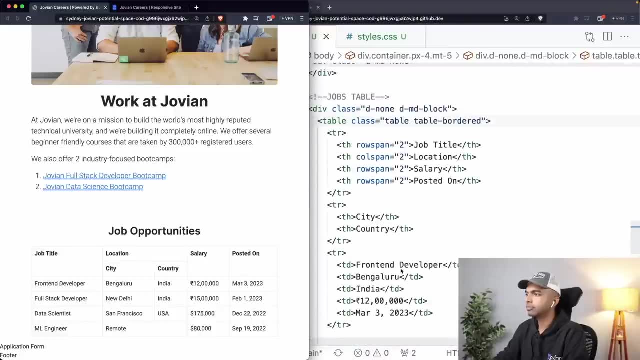 I think this would be nice. Let me copy this table striped CSS property. And this is how you work with bootstrap: You look at an example that contains what you need and then you just add that property, So, table bordered. let me add the CSS property: table striped. 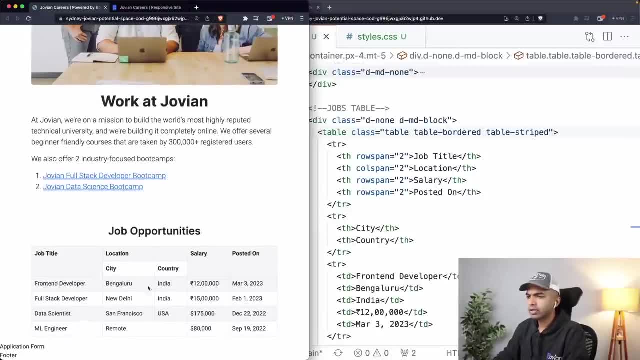 And, yeah, I think the table is looking nice. Okay, Maybe I can make a few changes to this, particular to the heading, because the heading, the header row, should probably look a little different. Let's see How can we color. How can we color the table. 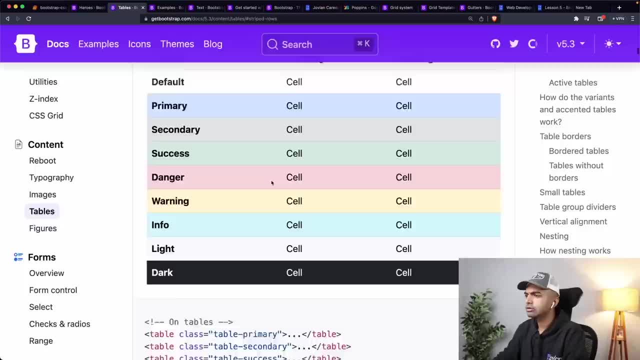 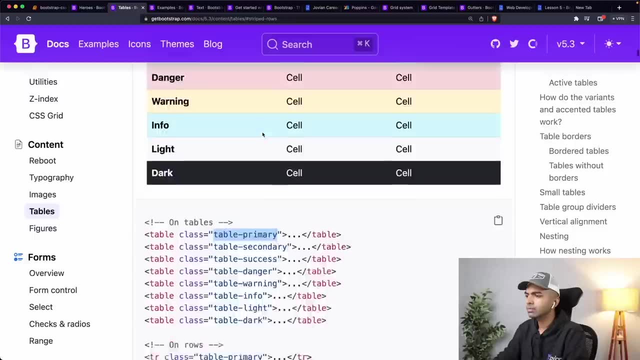 Are there any changes? Are there any colored tables here? Okay, It looks like there is a way to color tables as well. We can use this table primary class to give it a primary color, but I don't want it on the entire table. 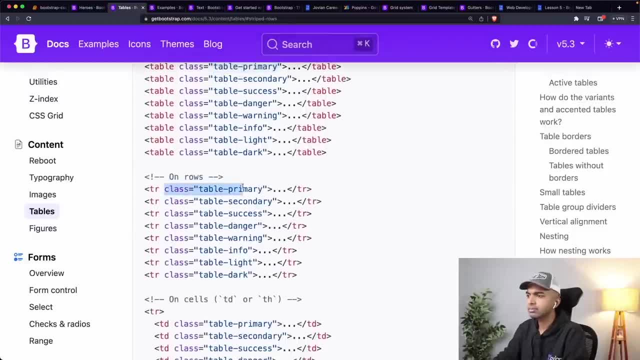 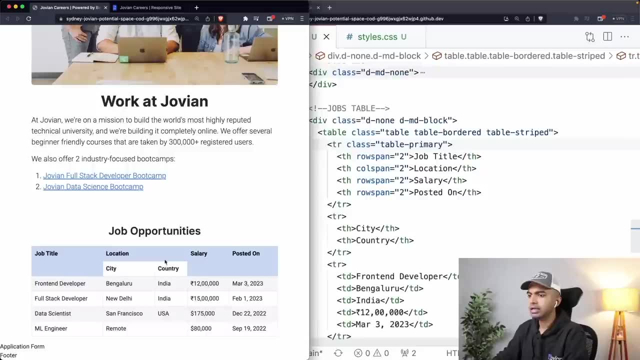 I just want it on the header rows So it looks like I can just add class table primary on a row and it should just color that row. Let me color the first header row, table primary. Okay, Nice It gets. it gets this nice primary color. 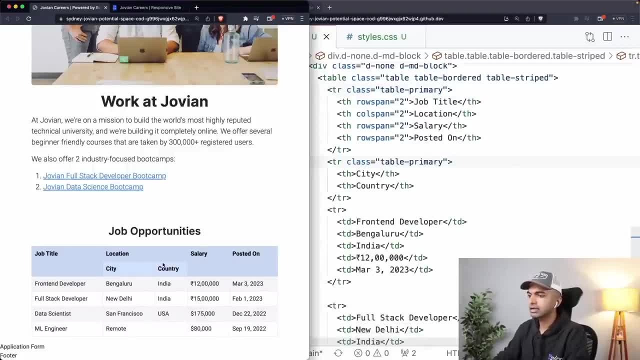 Let me add this to the second row as well, which contains the city and country, and this gets the nice color as well, And, because of the striping logic, this gets a slightly different color. Okay, Our table is starting to look good. 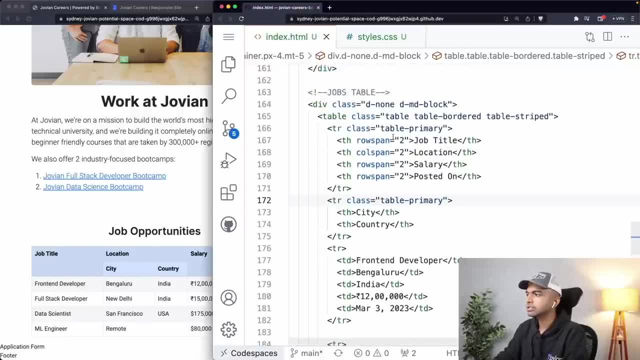 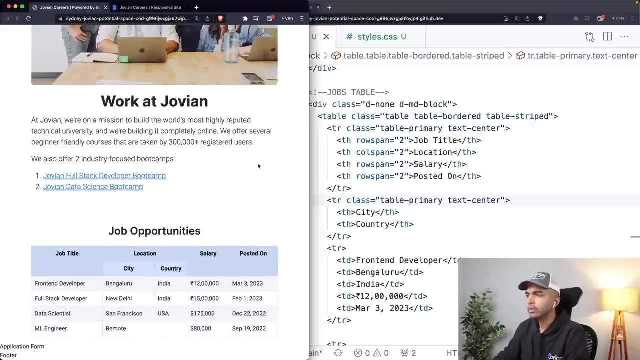 I think I want to center the titles here, The, so I'm just going to add text center or the table row, text center, Right? So this is how you build it out step by step. Okay, Nice, The table is looking good. 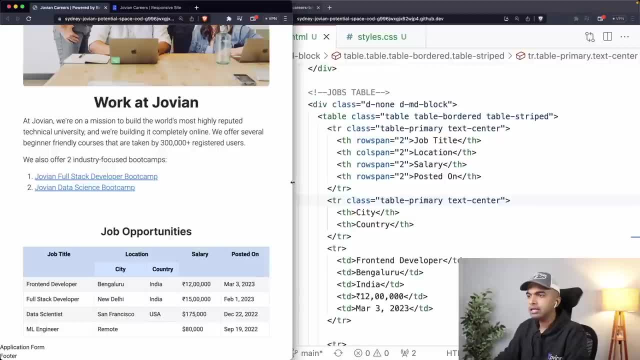 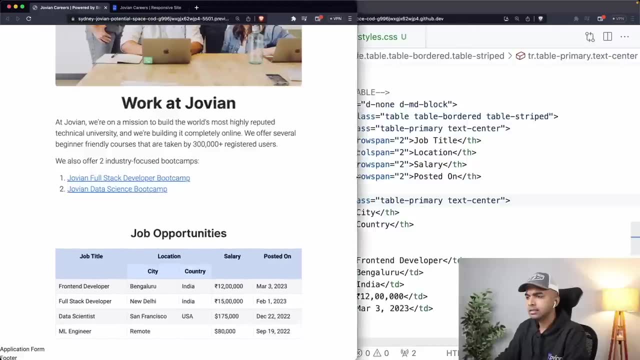 So Mobile, This is fine On MD. I'm going to switch into the table, which is looks fine to me. I think it's not. it's not cramped or anything. Okay, When we get to LG and higher, it looks like this is: this table is getting too big. 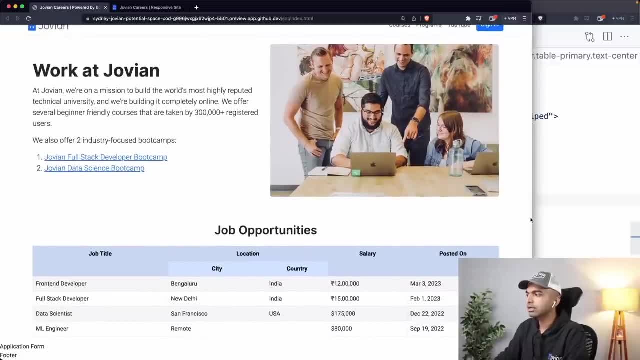 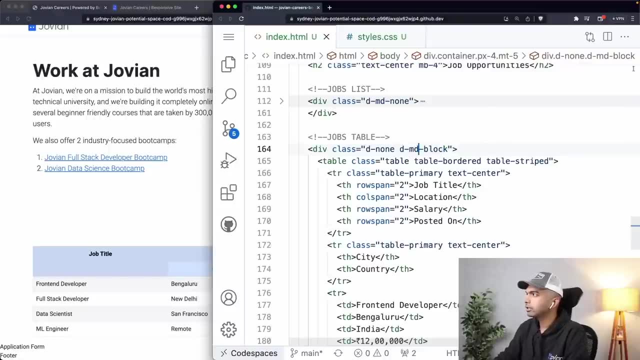 Maybe I might want to just limit the overall size of the table a little bit. So this is where I can maybe use a small helper layout here. So what if I do this? let's say, on LG. On LG, I limited to just eight columns instead of taking the entire 12 columns. I limited 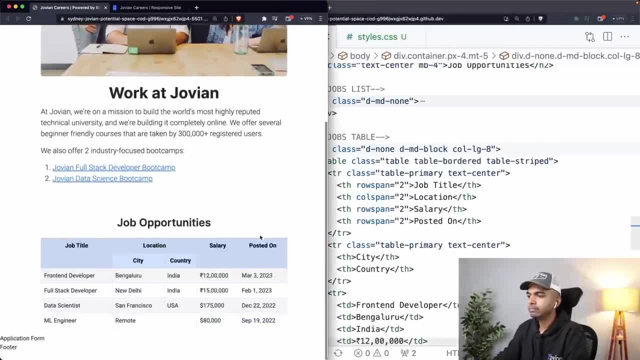 to eight columns. So on MD it's going to take up the full width which is here, but on LG it's going to just take up eight columns, But of course I don't want it to take up the left eight columns. 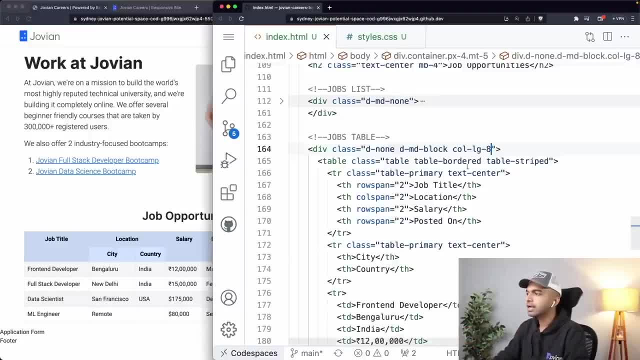 I want you to take up the middle eight columns out of the 12, but that's where I can add an offset, So I can say offset LG or maybe offset LG two. Yeah, So what I'm saying is leave two columns, Okay. 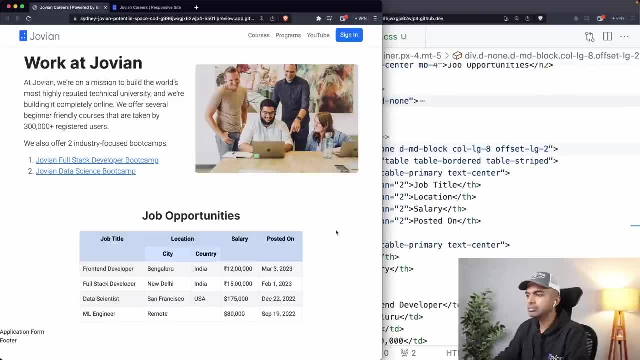 Okay, Leave two columns here. leave and then take up the eight columns, and that automatically leaves two columns here. 12 minus eight minus two is two, All right, So that way the table is going to be sent completely full width on medium screens, but 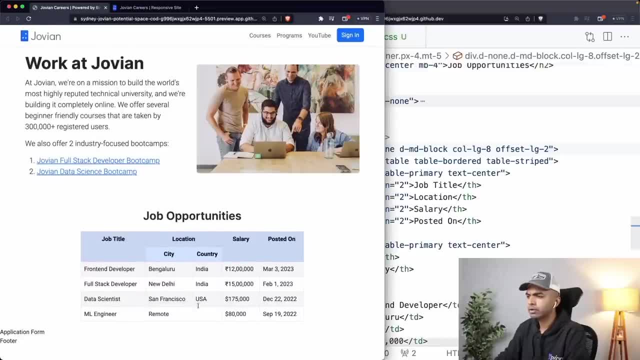 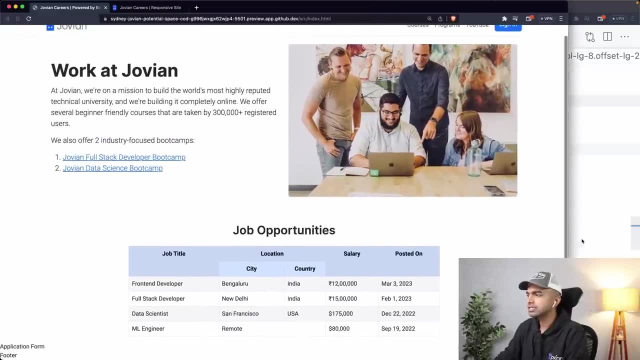 on large screens. it is going to simply take up. Okay. And last case, that is simply going to take up the eight columns in between, and that just expands a little bit, but it still looks nice, I feel. Okay, So that's great. 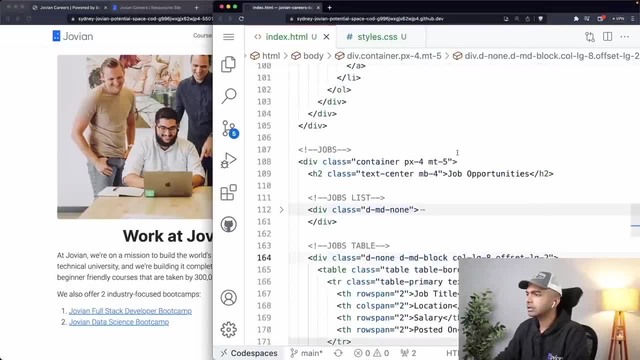 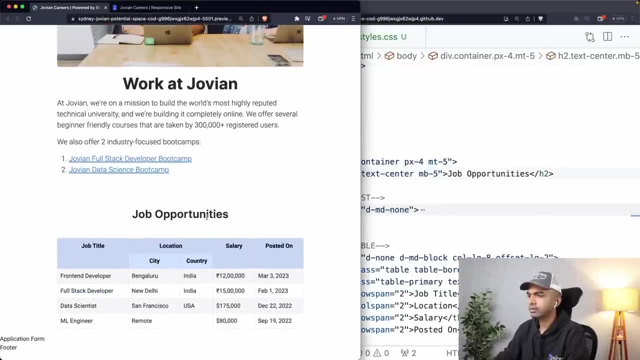 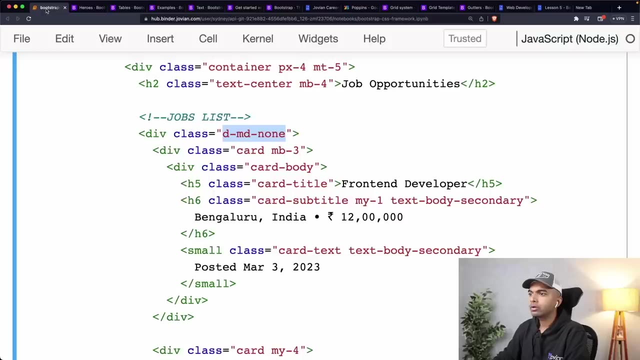 I think we've been able to set up a nice table. Let's see, maybe I can just increase this gap a little bit. MB five maybe here. Yeah, this is looking a little nicer. Okay, So our with that. we are done with our jobs list and jobs table. 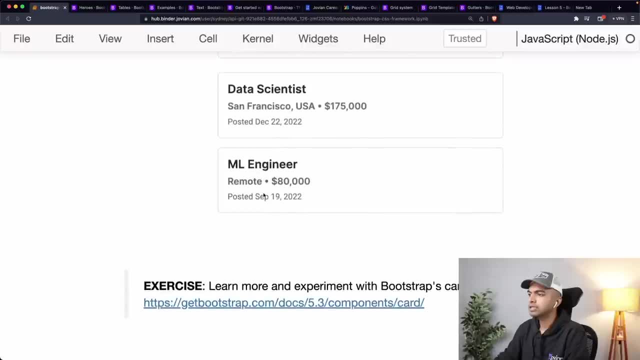 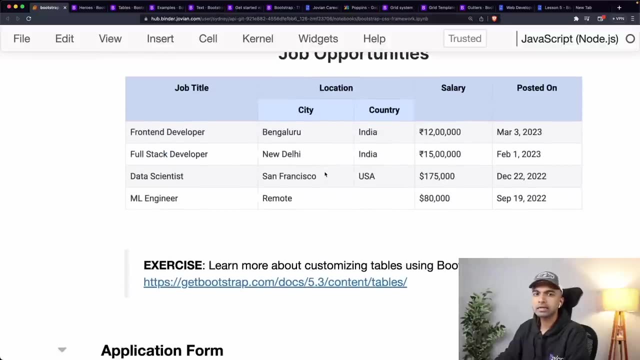 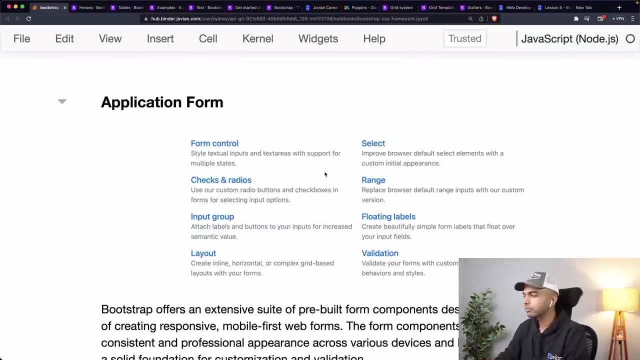 So this is what our jobs list looks like: job opportunities on mobile. And then we've also added a table, and this is what our job opportunities table looks like: Perfect. Next, let's move on to the application form. That is probably the only big piece that's left here in the footer should be pretty straight. 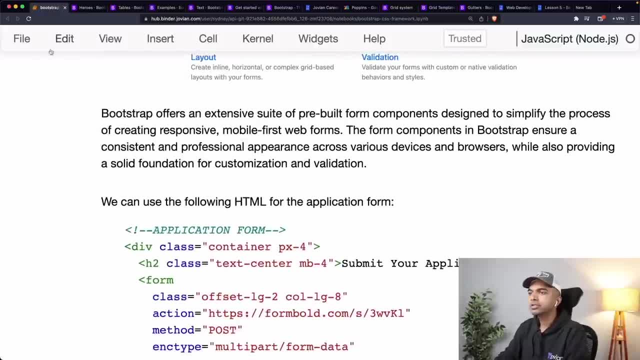 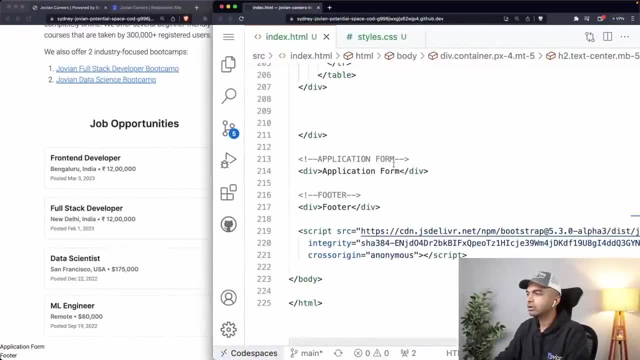 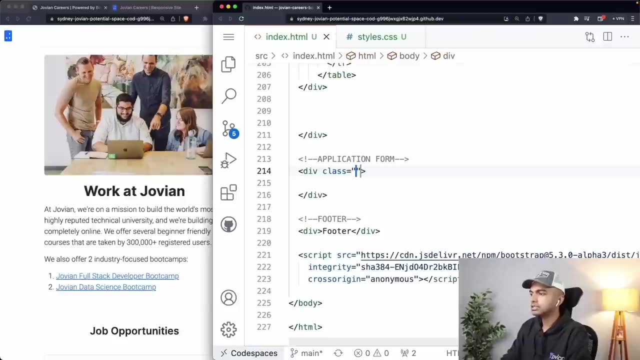 forward. Now for the application form. once again, bootstrap offers various pre-built form components. Okay, So first let us just set up the basic layout, and then we are going to start incorporating this one by one. So once again, I need a container here. so I'm just going to give it a class of container. 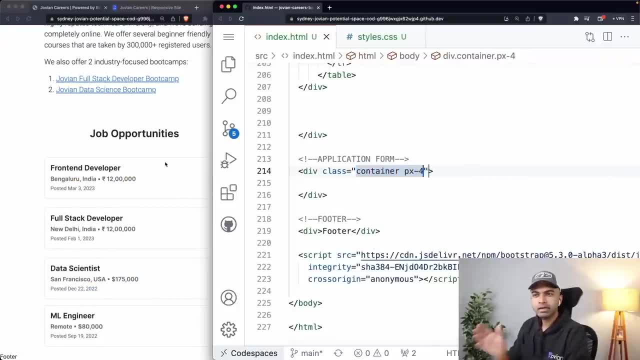 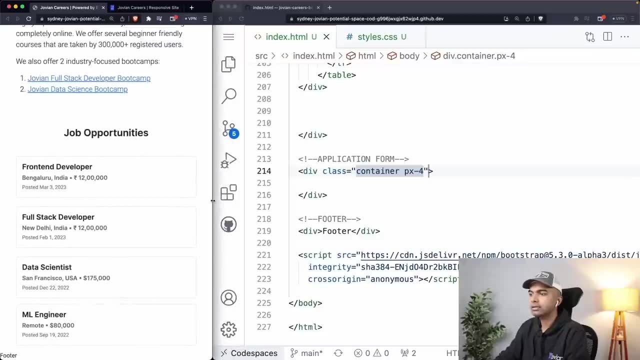 and PX four because I want some spacing left and right. So PX is the padding. It is basically this space that you see on the left and right. It's nice to have. I think it's it's good We can keep it. 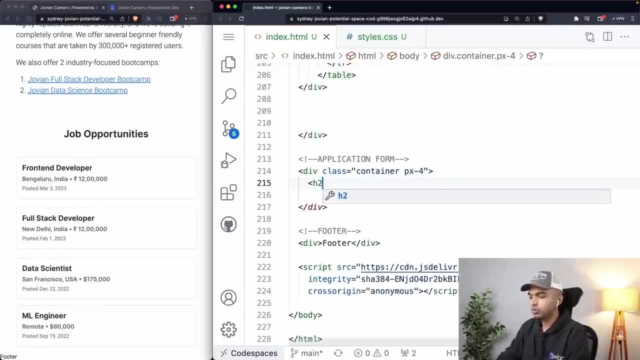 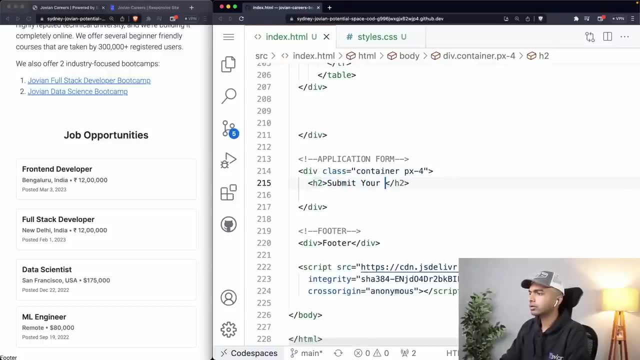 Okay, Then I need an edge to here, So H two, and in this H two I want to put in submit your application. Okay, The edge two is looking okay too. Well, maybe for this edge two I can add a text center, because I want to. 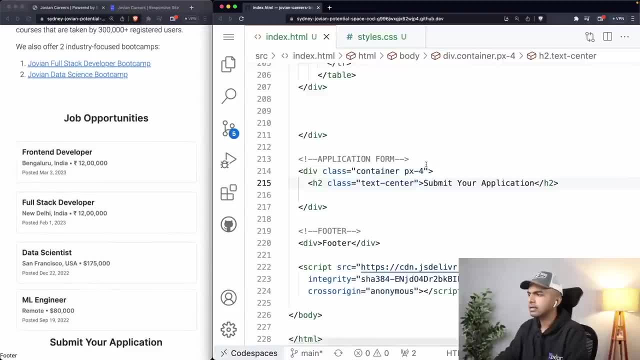 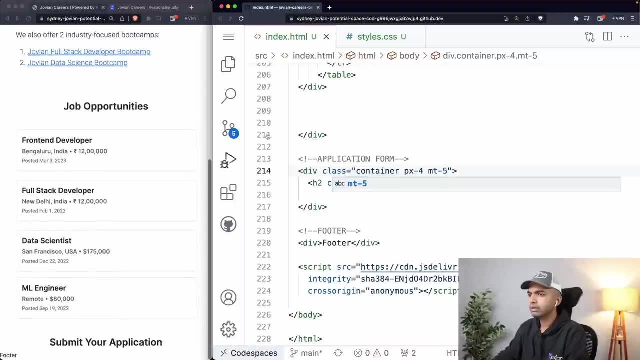 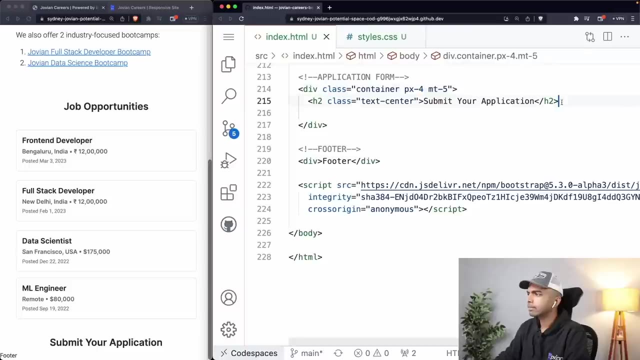 Center this text and maybe I need to add some space above as well. So maybe let me add empty five above. Okay, Now that has added some space above, and let me then also go ahead and add a form here. So I'm going to copy over the form that I had the last time, at least in terms of the 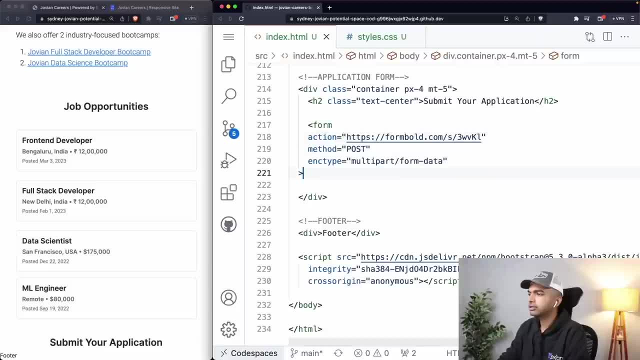 basic action and method. So remember we were using a tool called form. We wanted to actually post the form. Let me add the form element here. Okay, I've added the form and now into the form I can start adding inputs. Okay, 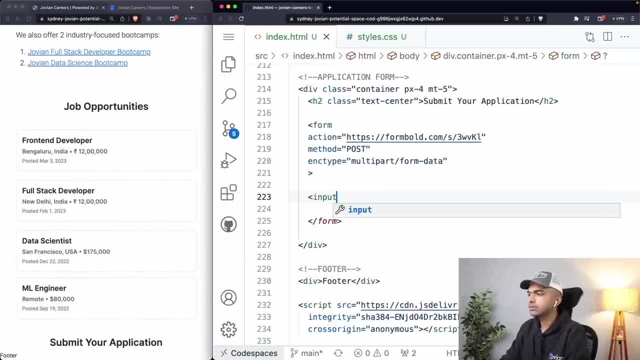 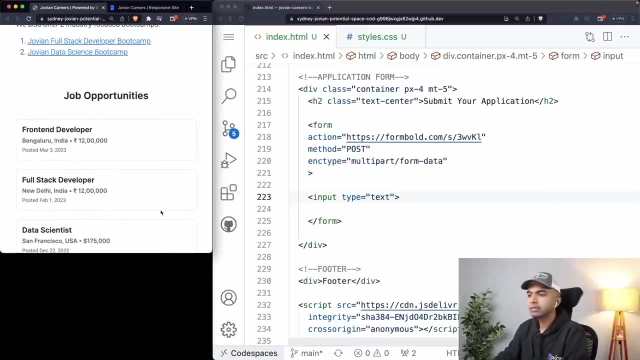 So I've created a form, but this form doesn't have any inputs yet. I could put like: input type equals text, and that should create an input box here. So let me just move this up a little bit. You can see that now I have this input box. 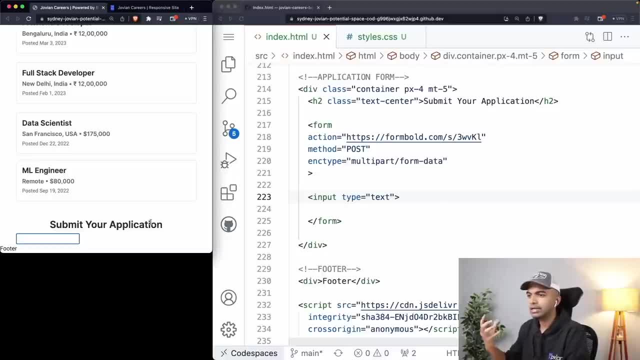 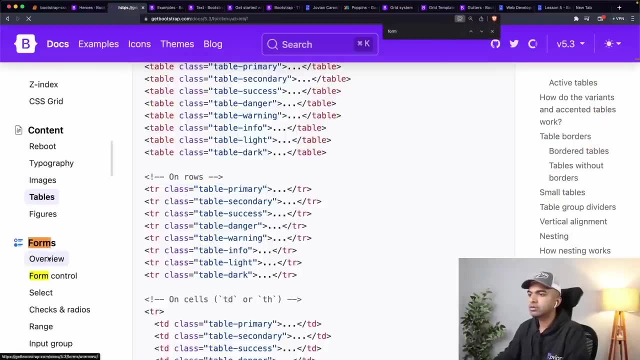 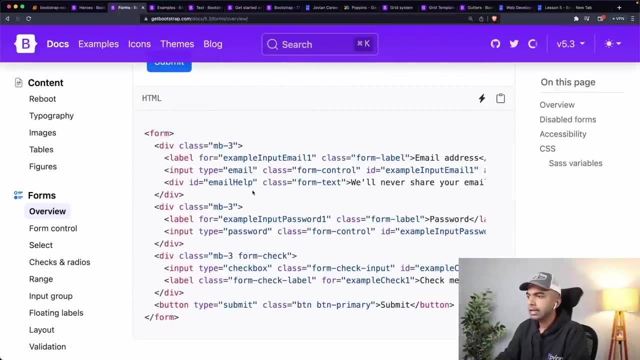 But of course, I want to use a nice input form that is created very nicely with bootstrap. So I'm going to come into bootstrap here and I'm going to search for form. Okay, So here is an example of forms. Looks like you don't need anything on the form component and for the actual inputs. 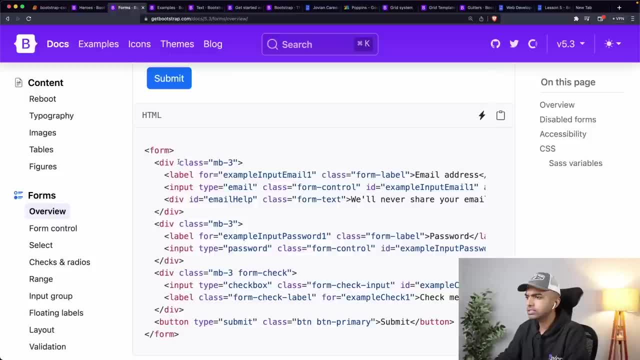 looks like we need to do a bunch of things here. We need to set a class of- okay, this is just a. we need to put the input and label and maybe some help text in a div And we then need to maybe specify the class form label for the label. 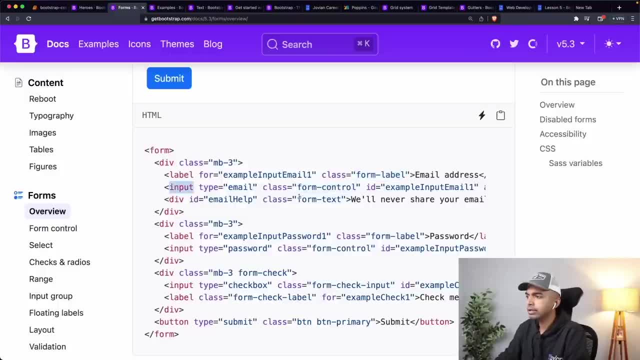 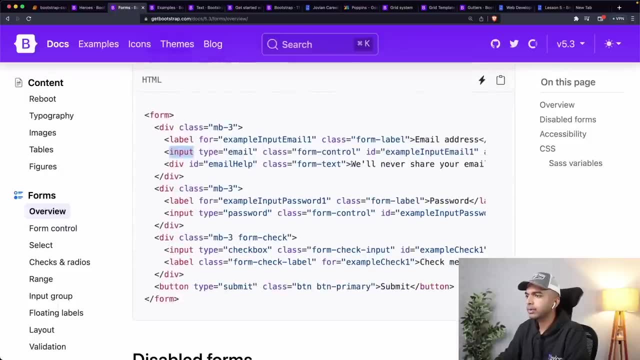 We need to specify the class form control for the input, And if we want some helper text- so this is some helper text that we want to show below the email- then we can specify some helper text as well. So how about we simply copy this over? 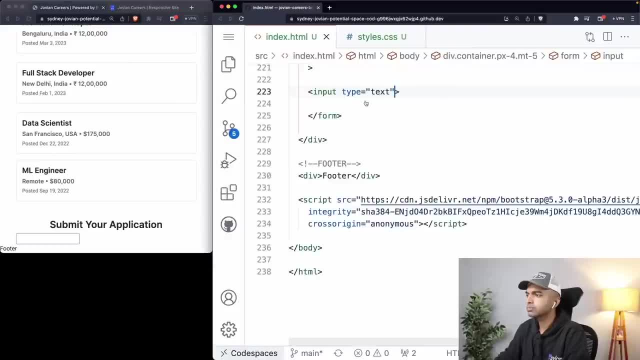 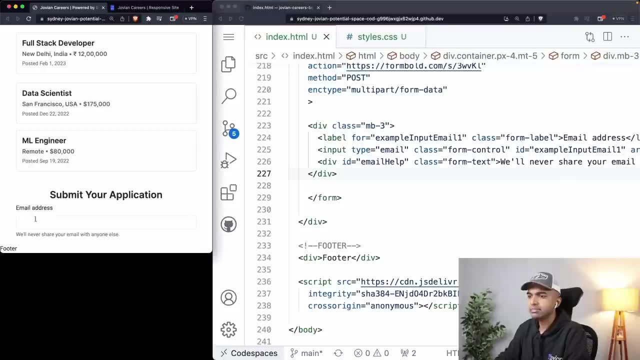 I think we understand this well enough so we can just copy this over and let's put it into our form instead of this: Okay, All right, So just like that. We have this email address Input field. that is looking good, And I am going to simply give it the. I'm going to give it the ID email. 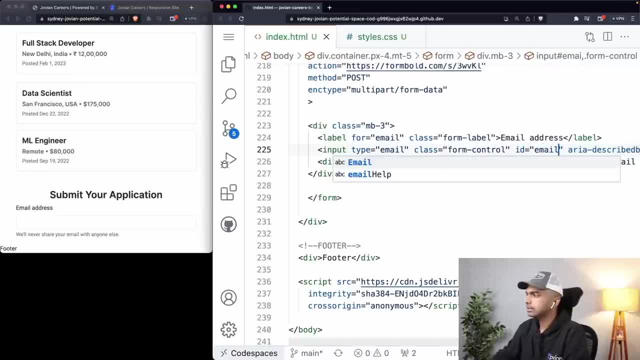 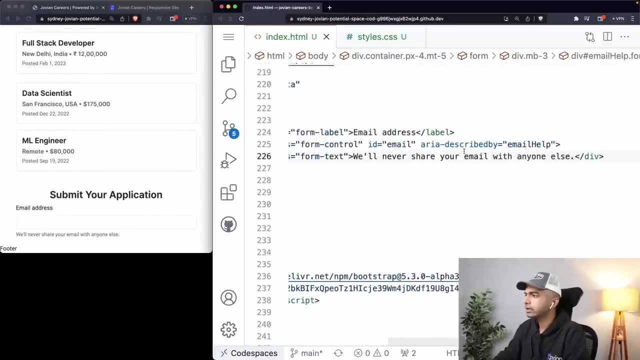 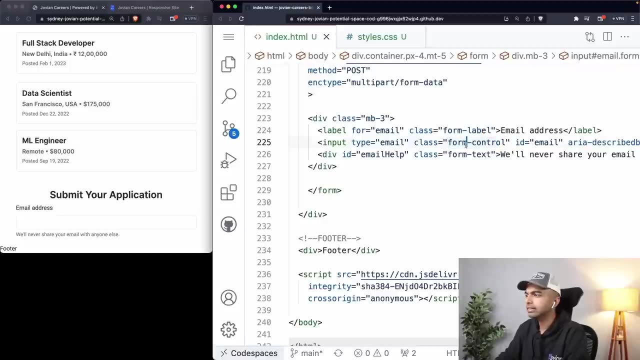 So the input is going to have the ID- email and the email help is the description below the email address. This looks fine as well, And, yeah, I think this looks good. So we need form label and form control. It looks like these are the two things that we require and that automatically helps us. 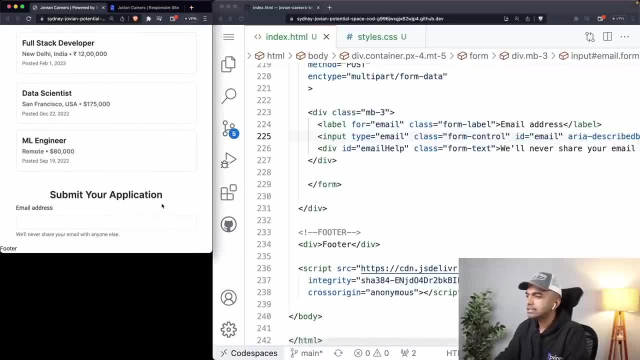 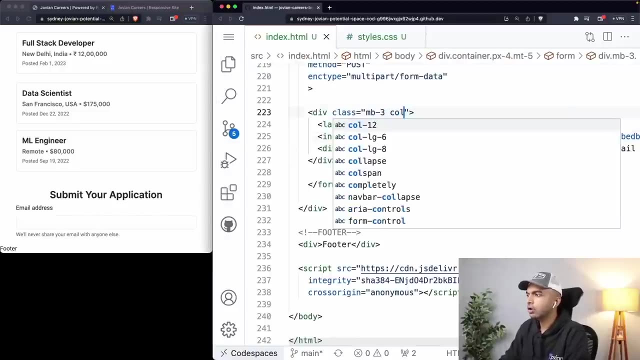 create the layout. Okay, What else? Well, I feel like maybe we don't want to use the entire, We don't want to use the entire width for email of the page, Maybe we want to use just maybe half the space. So I can go in here and I can say: call six. 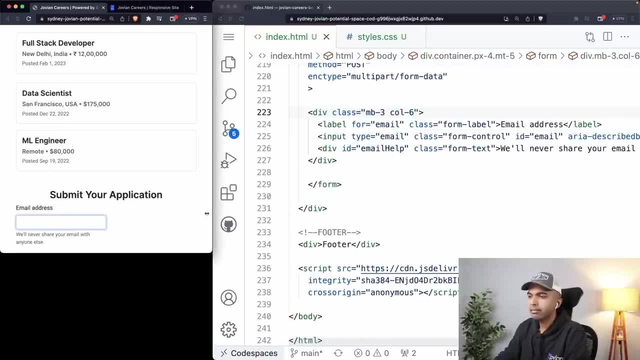 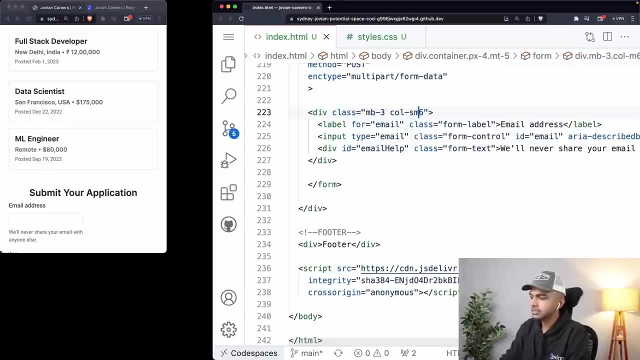 And this way it is only going to take up half the space. But now the trouble is: even on a really small screen it takes up only half the space. Let me say, call SM six And this way, on a really small screen, it's going to take up the entire width. 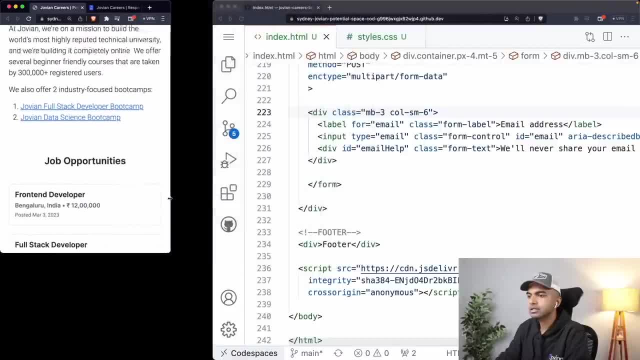 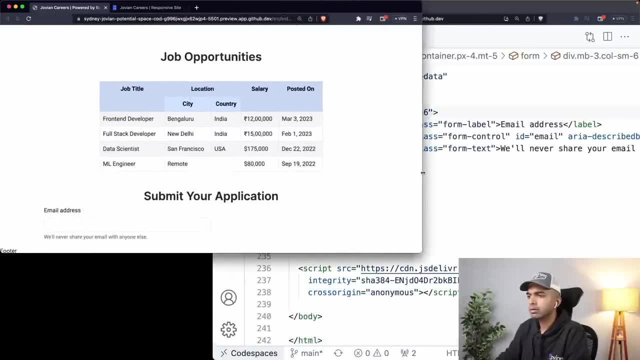 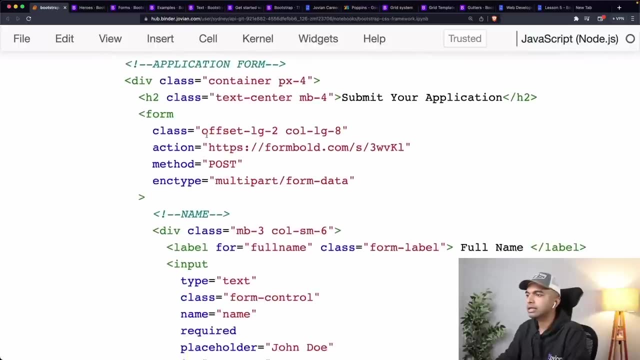 And then, as soon as we enter bigger screens, it's going to take up less width. Okay, So this is good. I think I'm happy with this. Okay, Perfect, So just like we have email. I have also already put together some other examples. 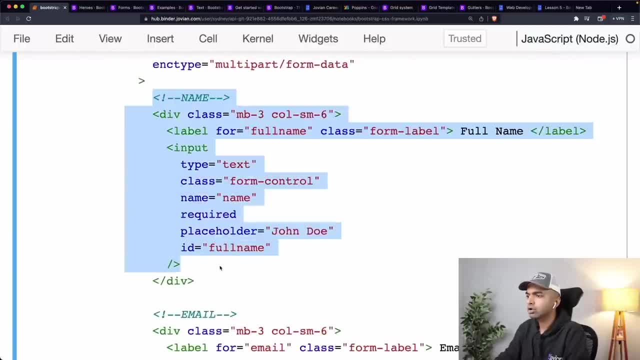 So here now I have this name field, So I'm just going to copy the name field. All we have is we, exactly we have the exact same MB three, Call us, I'm six, except this time the ID and the name are full name or name, I guess. 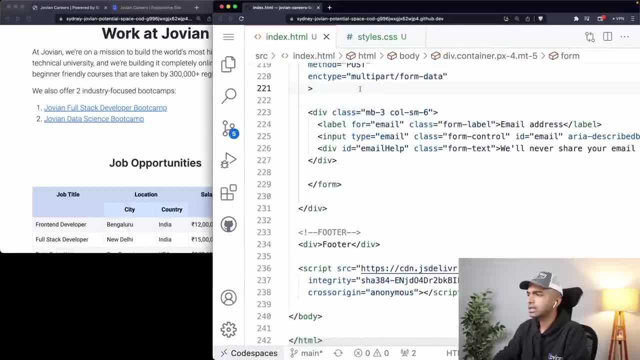 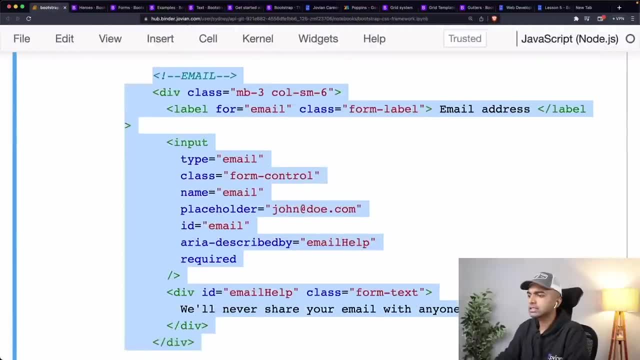 So let me just copy this over, and this is of type text. So let's insert the name field. That's giving us the name field email. We already have the email field, but let me just in any case, copied over once again. 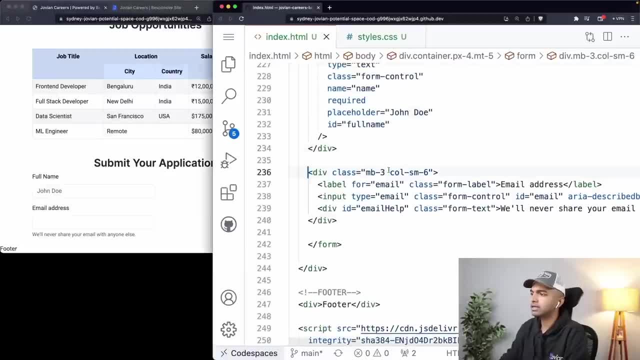 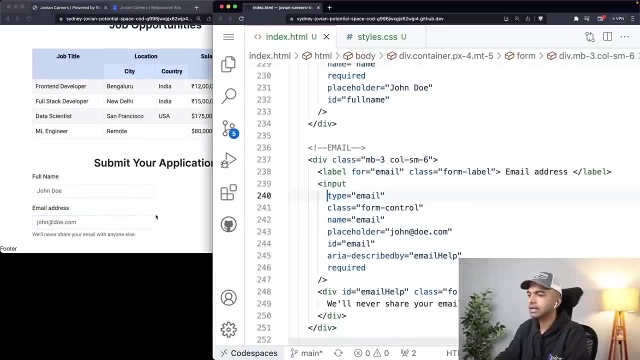 So that is going to give us the email field. The only difference between the name and the email field is, of course, their ID and name are different. the field name, but also that the type is email. Okay, So automatically add some validation. and we've also added a placeholder and we've added a. 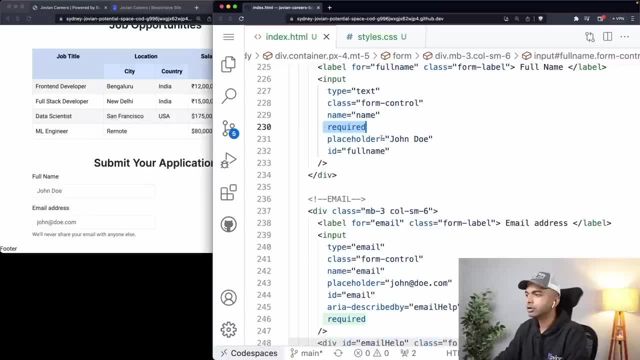 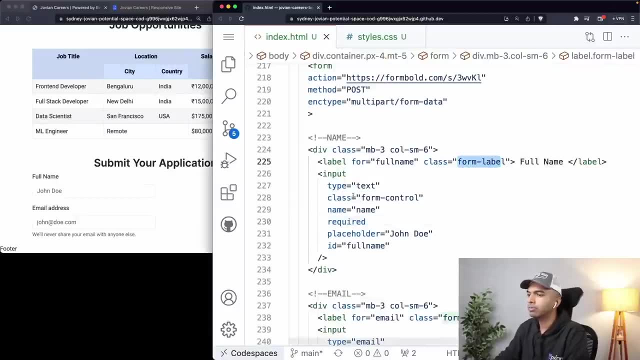 required field. So forms: we've covered in a lot of retail already, So I'm not going to go into the specifics here. but now we have the name field, We have the email field. All we've done is I did a few bootstrap classes- form label and form control, which makes it. 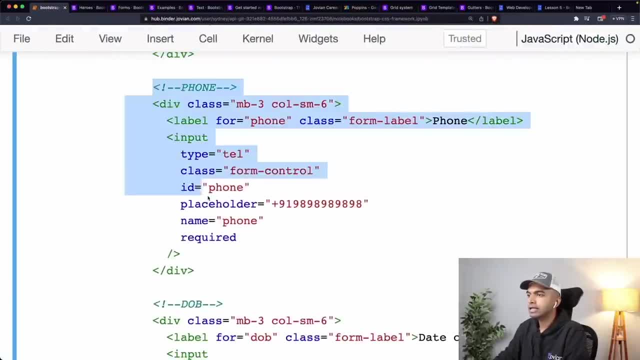 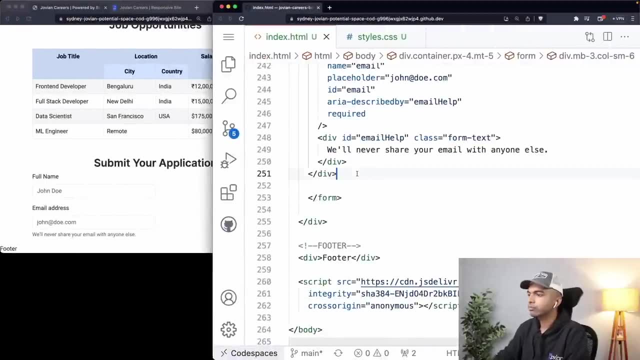 look nice, Let's get the phone number field. So again, the only difference here is the titles, labels, IDs, and the type is T, L, tell, which requires this to be a phone number field. Okay, Okay, So I'm going to add the document a bit. 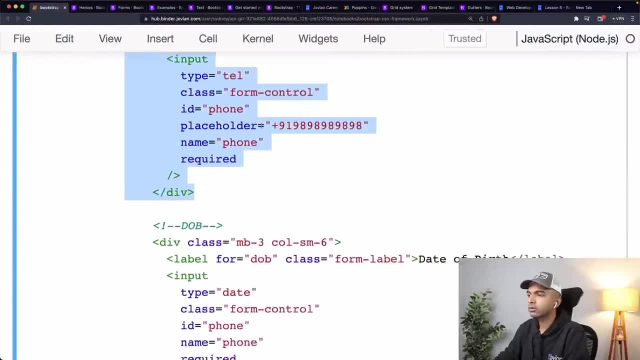 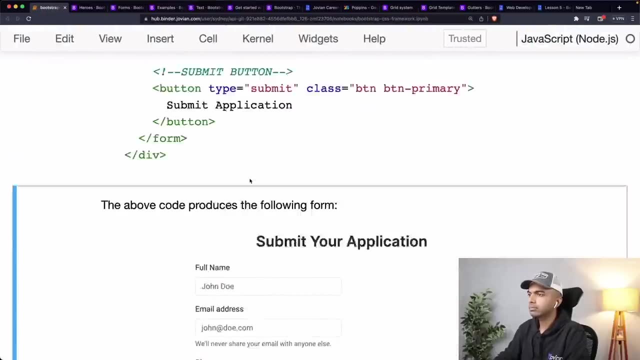 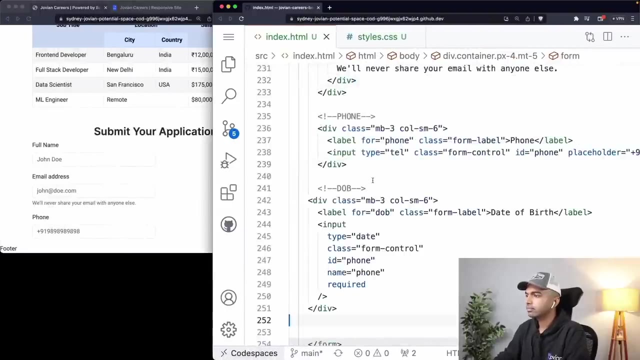 Yeah, Cool. So now we have the phone number field as well. This is looking good, Let's get up there. Let's get the date of birth field as well. Okay, Let's get date of birth. So yeah, but date of birth we have. once again, we have the same layout, exactly except that. 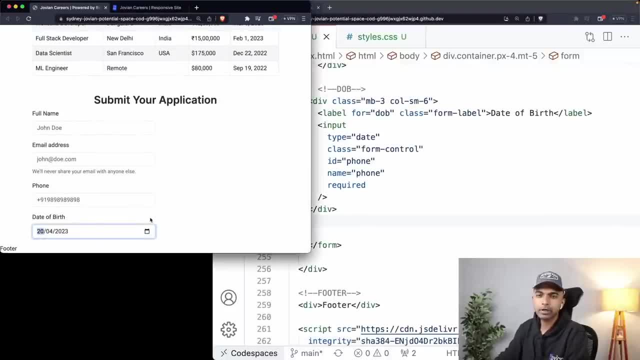 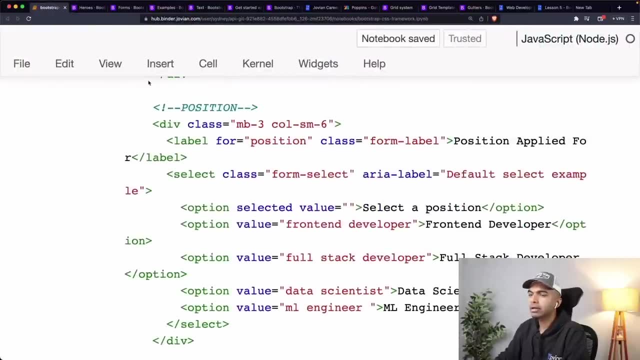 this time it's a date picker, So you can go in and you can actually select a particular date here. So that's good, Okay. Next up, We have apply to field, So this is more of a dropdown. This is like a select component. 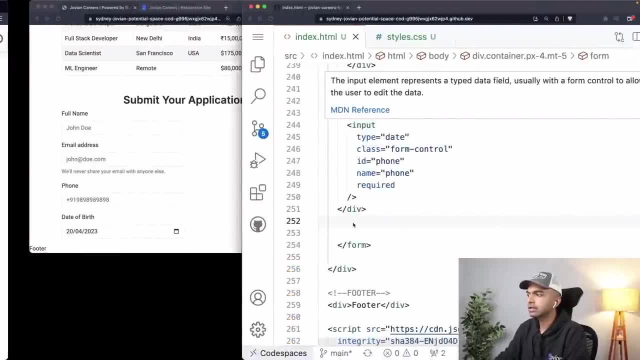 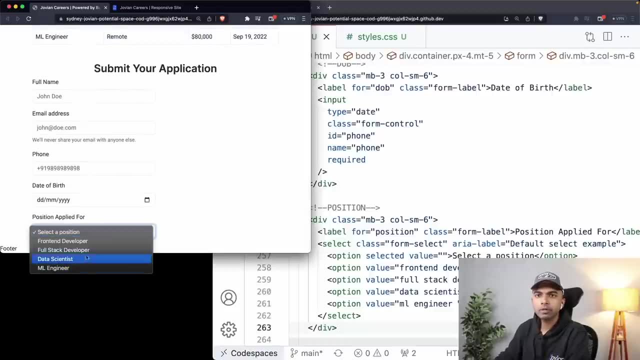 I'm just going to bring it in here first, So the position applying, and then we're going to look at it. take a close look at it. Okay, So the position applied for is a dropdown And from here you can select whether you want to apply for full-stack developer front-end. 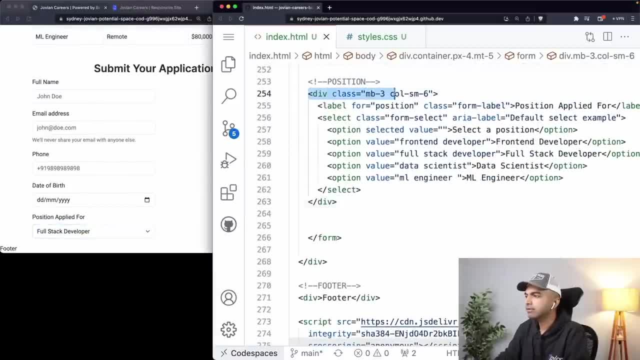 developer, et cetera. So how are we doing this? Well, once again, we have class MB three and call SM six. Now, the only difference here is, instead of an input, we're using a select, which is what we have to do. 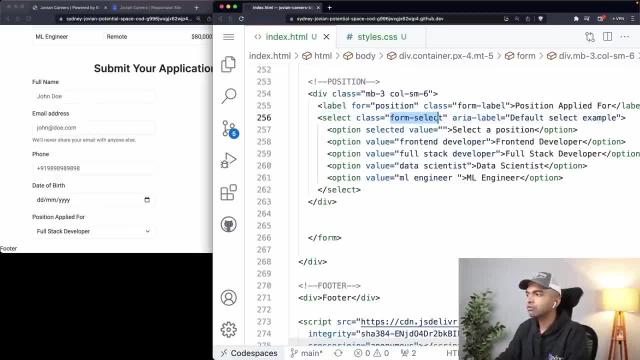 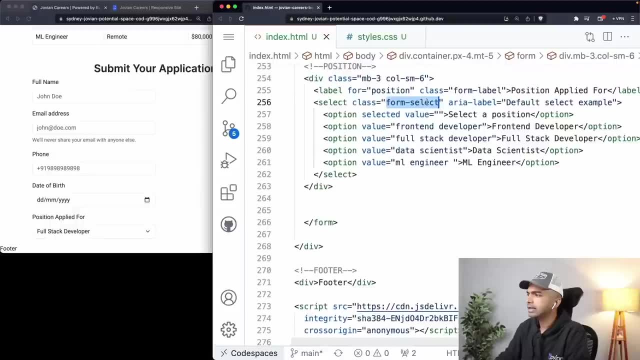 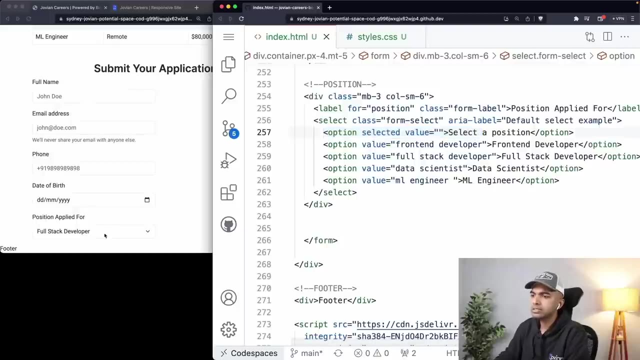 Anyway, but the class we are changing now from a form input to a form, So it was called form control here. Now that has been changed to form select and that's it. That's the only change. The label still says form label and we have a default option with an empty value set to. 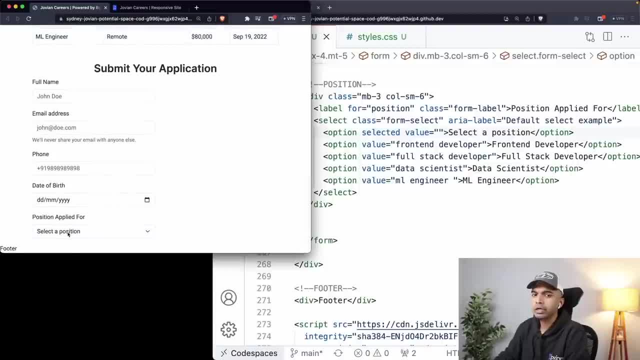 select a position. That's why, by default, it is pointing to select a position, And we have then a front-end developer, full-stack developer, data engineer, ML engineer. If you want to do a full-stack developer, you can do a full-stack developer- data engineer. 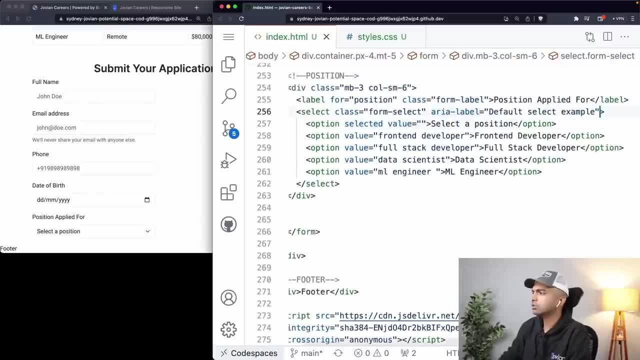 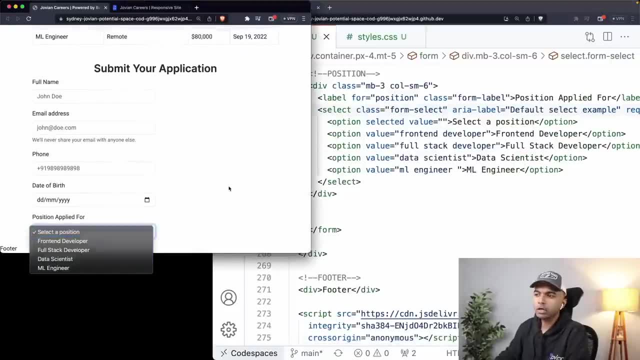 ML engineer. If you want to do a full-stack developer, you can do a full-stack developer, data engineer, ML engineer. But typically we can also make it required So that the user has to select a particular option. So yeah, this is just a normal dropdown. 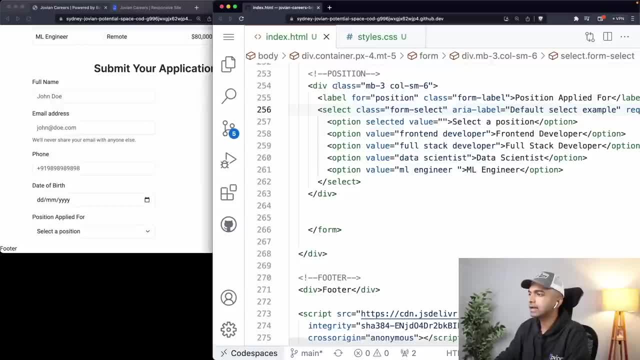 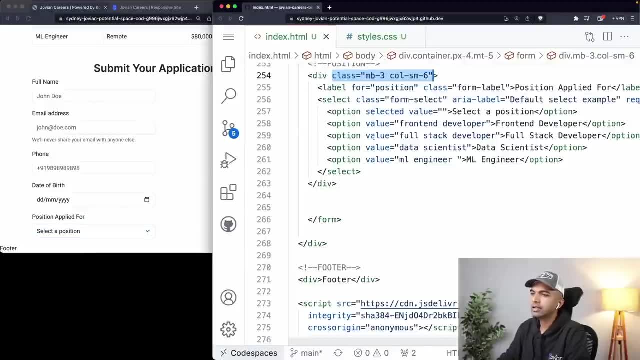 All we've done is added a class to the label, added a class to the select and added maybe this layout or this bottom margin and this six column layout here, so that it looks slightly nicer. Okay, Then we have this resume upload. This is a file upload. 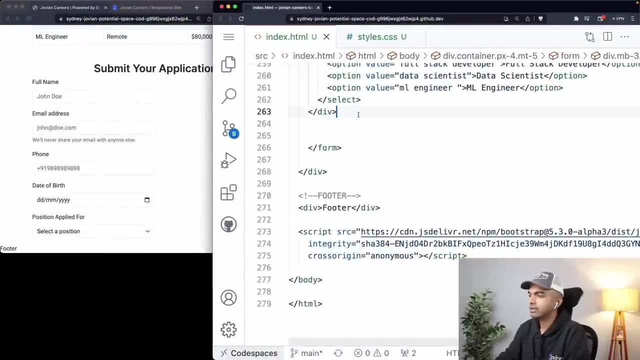 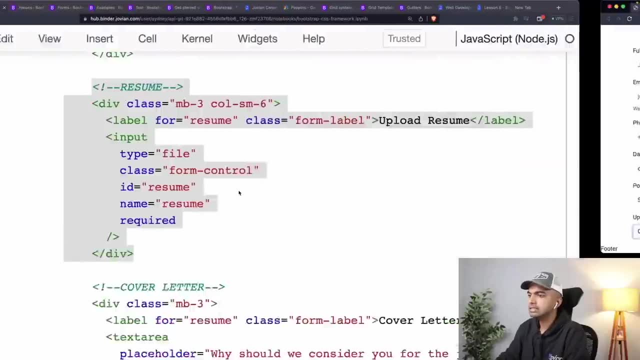 And the only difference here is that input type is file. So again, I'm just going to kind of bring that in directly As well. So here is your file upload and that allows you to pick a file. again. exactly the same. Finally, we have this cover letter, and in this case it is a text area. 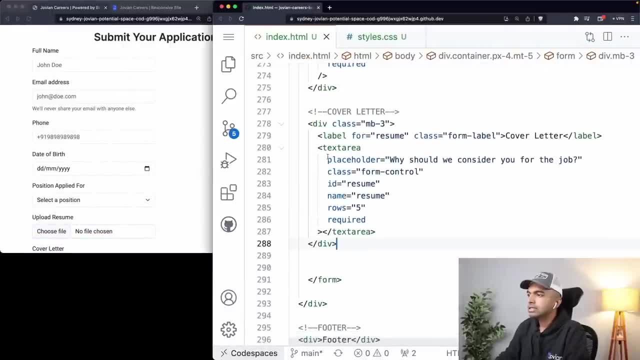 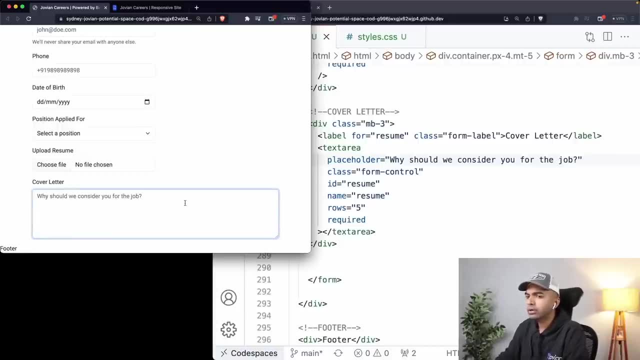 Okay, So no change here. Again, the only change I'm making is I want the text area to actually be full width, right? So I want the text area to be. I want the text area to actually be full width And that is why I've said I've removed that. call SM six. 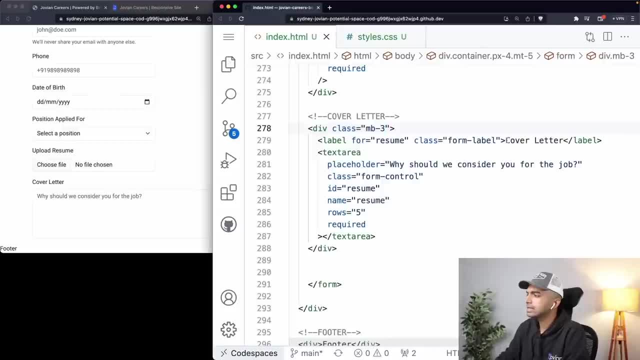 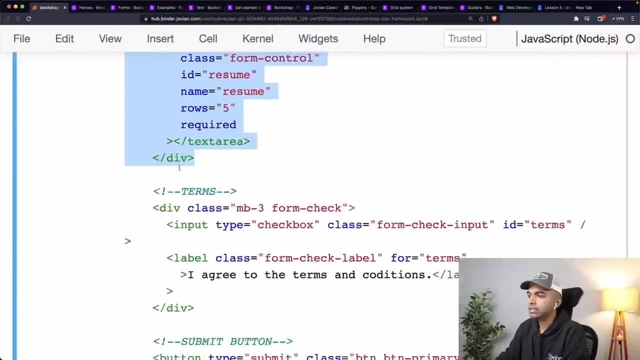 So I'm going to use a full width text area And that has a label, cover letter, And once again you give it the class form control And that's it. We have our application form. The last thing we have is the terms. 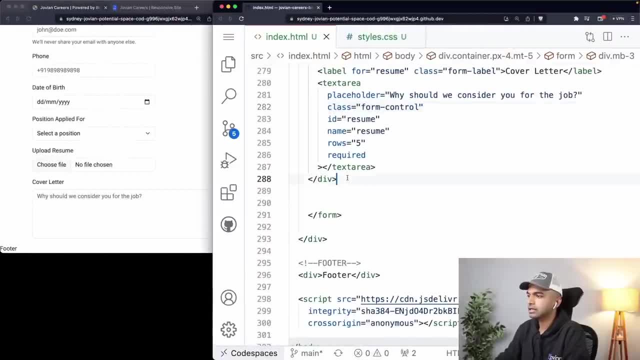 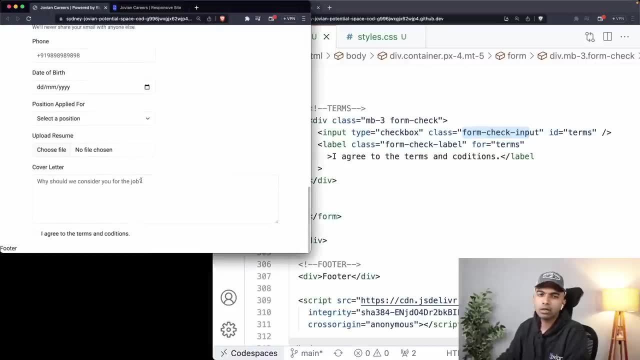 I'm just going to bring in the terms real quick, really straightforward. It's just a simple checkbox. So all we do is we say form check input and form check label Again. all this is borrowed from the bootstrap documentation, simply copied over and with. 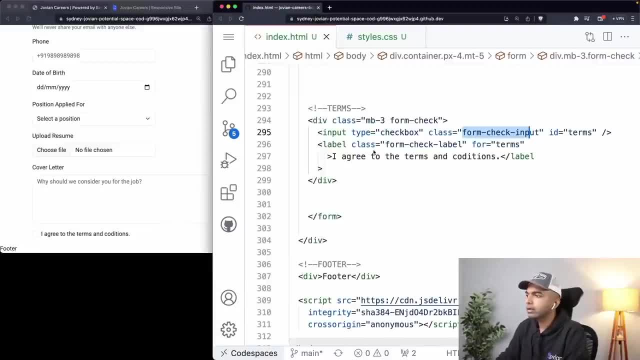 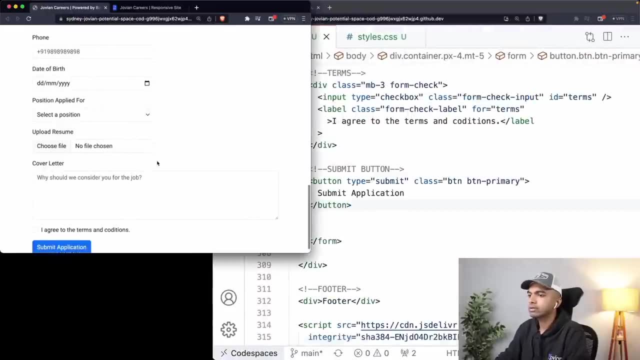 a quick assessment of how things are. What else? Um, There's a submit button right here, So let's grab that submit button. That is going to be a primary button for us. So we have submit application and now we are ready to submit the application. 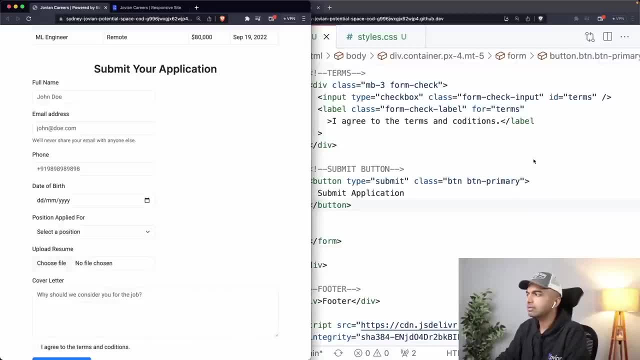 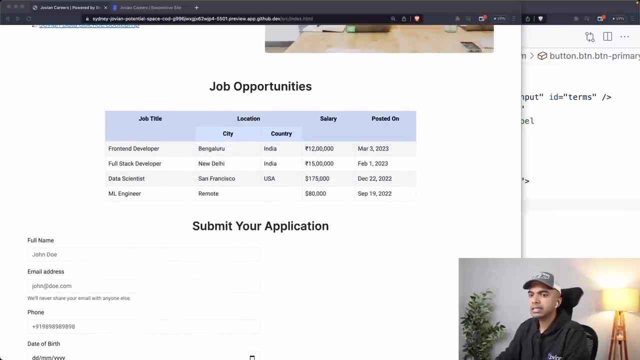 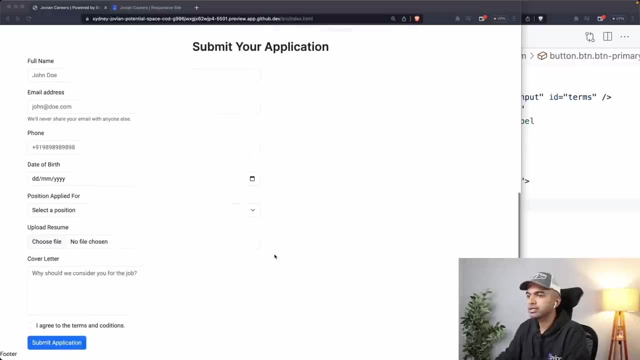 So that's it. I think this form is looking good. Maybe we can make like some final changes here. Let's see. Okay, I think the form goes. I guess the form goes too wide. I think we want to restrict the form to just be just as wide as this job opportunity stable. 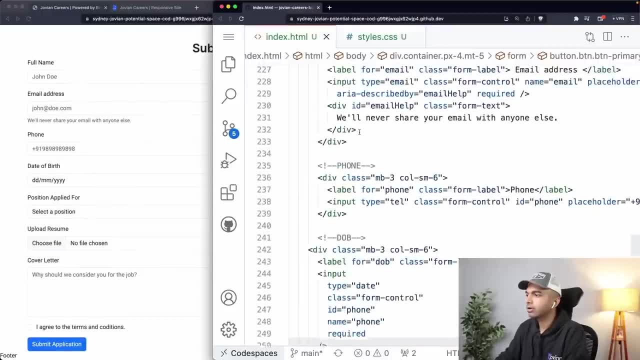 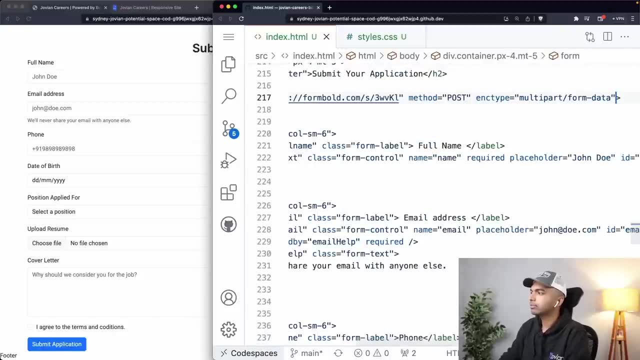 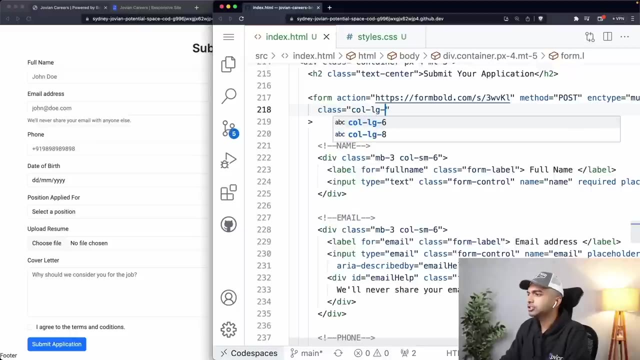 because otherwise it's going to become a little hard to actually Actually read the content of the page. So I'm going to add the exact same classes here that I had for the previous one. on the form, I am going to add the class LG. let's see, call LG eight so that it is not too wide. 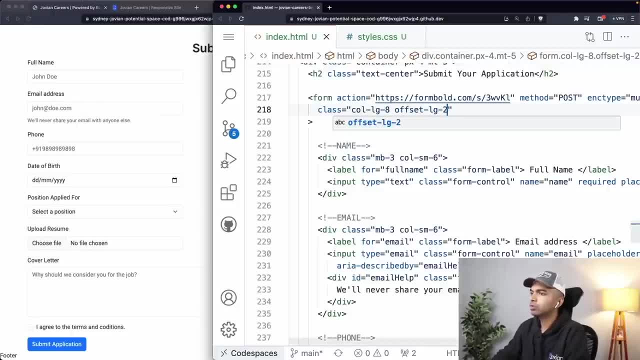 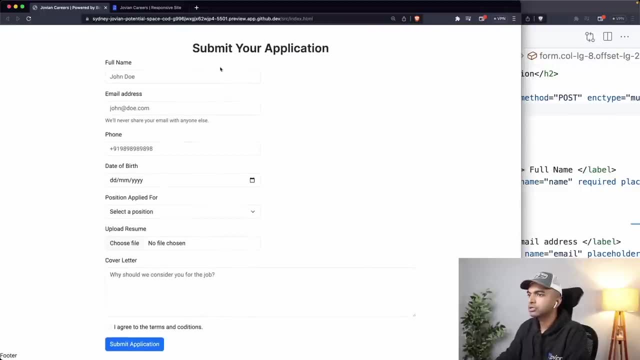 And I'm also going to add offset LG too, so that it is, relatively speaking, centered on the page. Okay, So now we have worked at Jovian job opportunities, Submit your application And we have the form as well. Let's quickly verify the form. 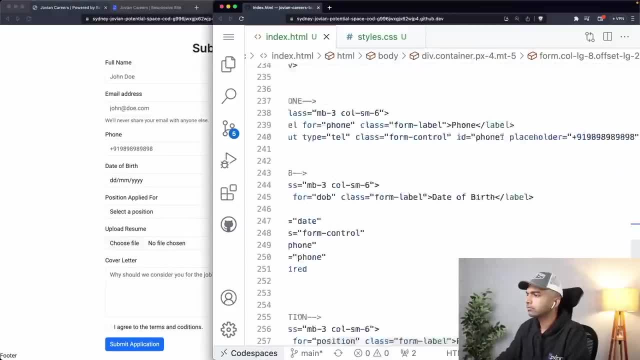 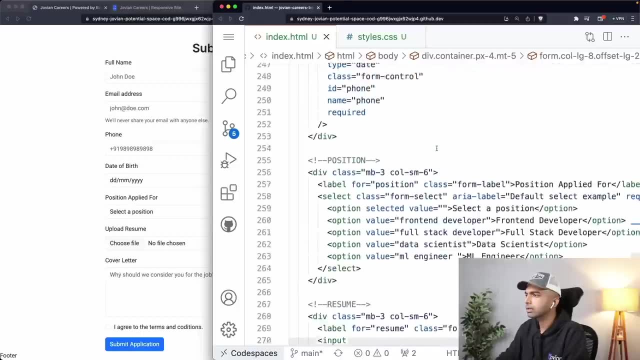 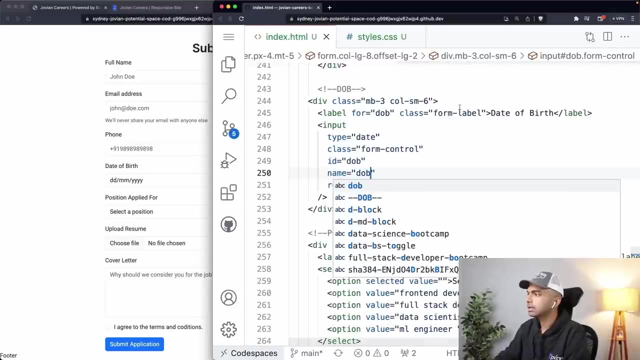 Okay, We have email. we have phone. Okay, Phone looks fine. We have date of birth. We have position. Yup, I think this is all. Let's check date of birth. Yeah, I guess date of birth needs to be changed to DOB. that changes to DOB, DOB and yeah. 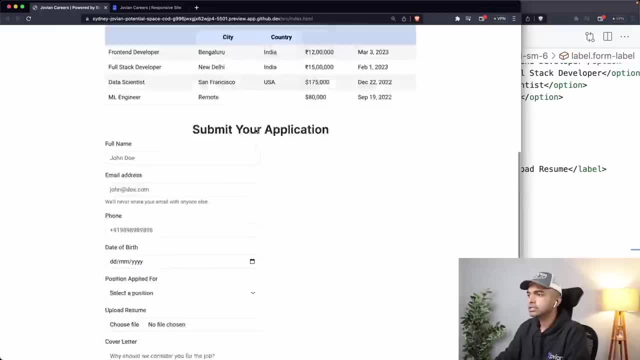 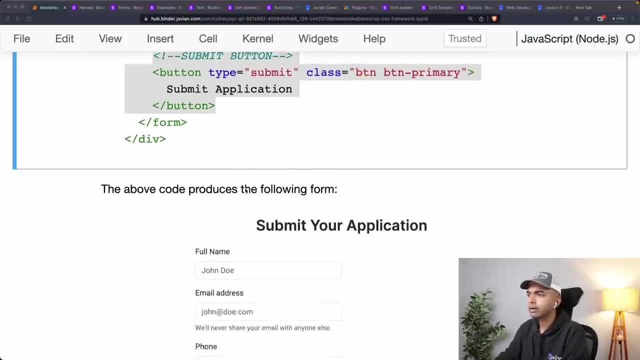 with that, our date of birth is fixed as well. Perfect. So now we have the form, Now we have the hero section, We have job opportunities. The final thing that we need is the footer. Okay, Now, where do you get the footer again? 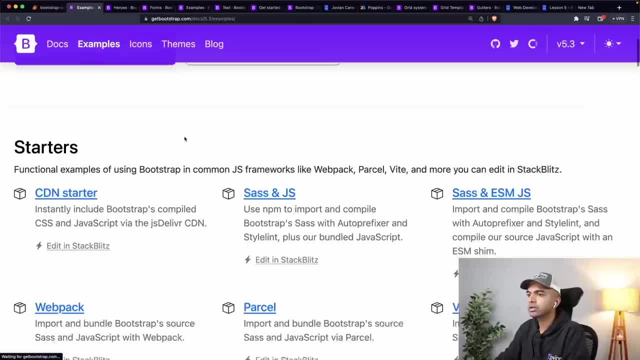 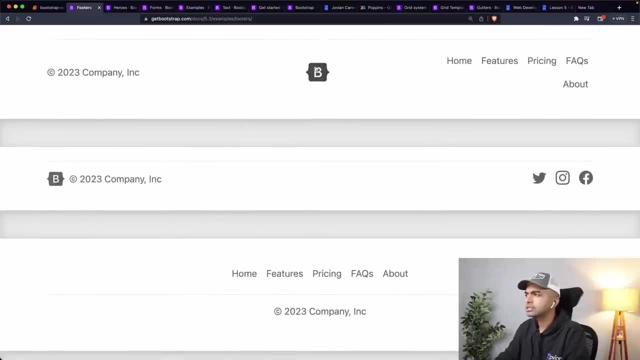 Bootstrap has a bunch of examples that you can choose from, So here are some examples for the footer. Let's look for footer and let's open up the footer. Okay, So there's this example right here. This is something we could do, or we could do something like this: 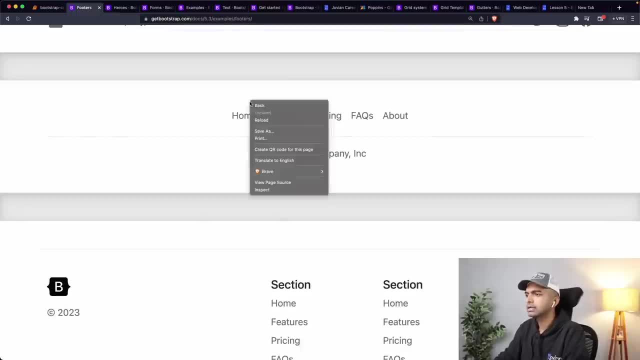 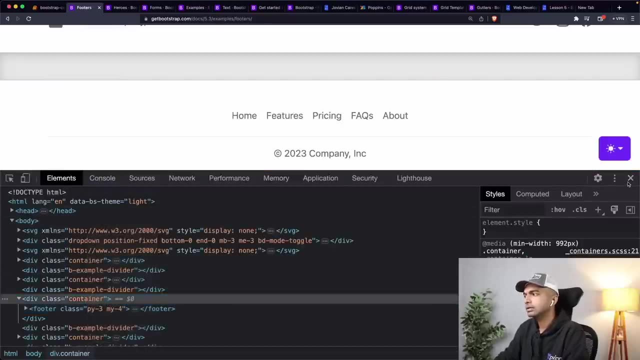 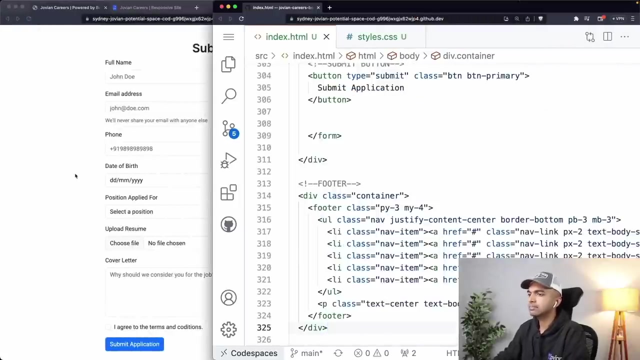 I think this might work out fine for us. So we could probably just right click, inspect and copy this entire container. Okay, Paste it in and make some desired changes to it. So I can get rid of this. I can simply paste that in and then I just need to make the desired changes to it. 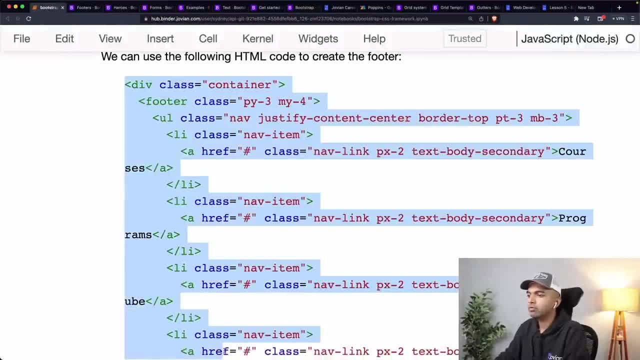 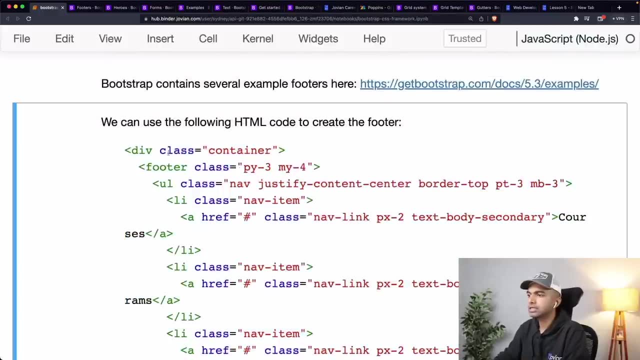 And because I made these changes already, I'm just going to copy it over from here. It's exactly what it looks like. I'm just taking an example of the footer, which is a container, and then it has maybe a PY MY and it has the list of links. 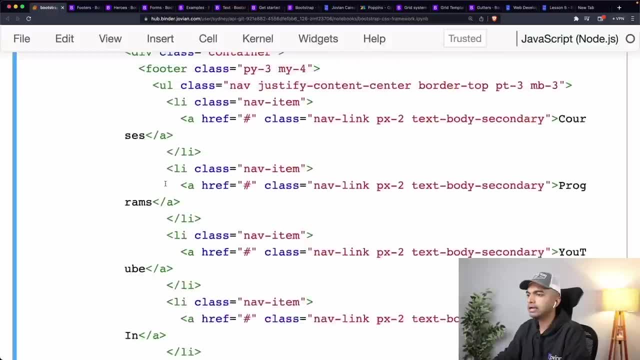 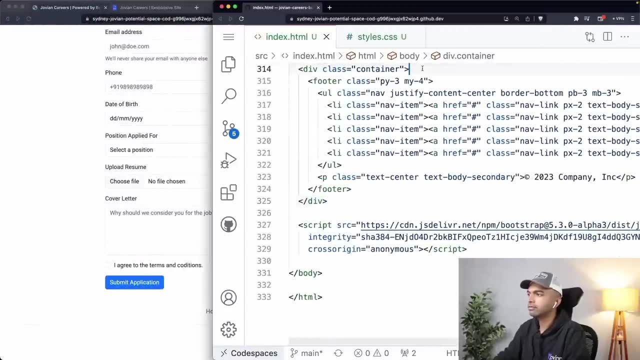 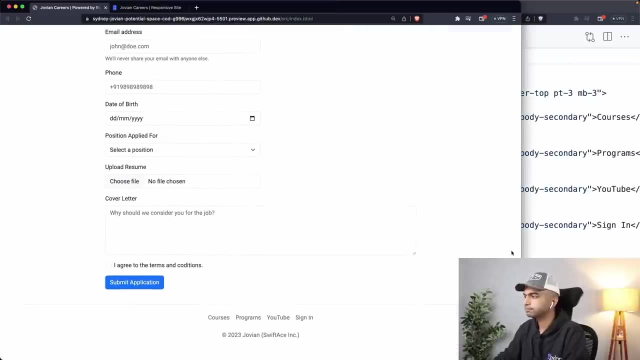 Okay, And below it it has this copyright text. It's a very simple, straightforward footer. I've just made very minor modifications to what we already have in the bootstrap example. Okay, Let's paste in the footer here as well, And with that we have a footer. 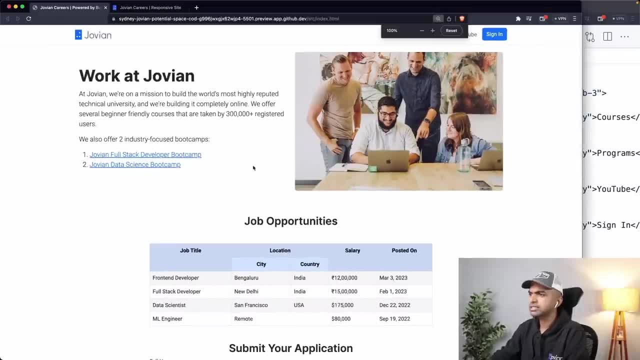 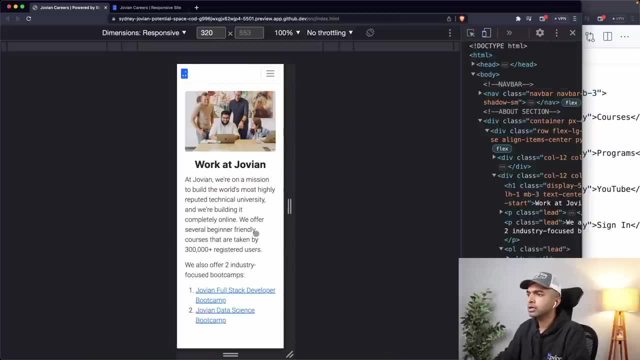 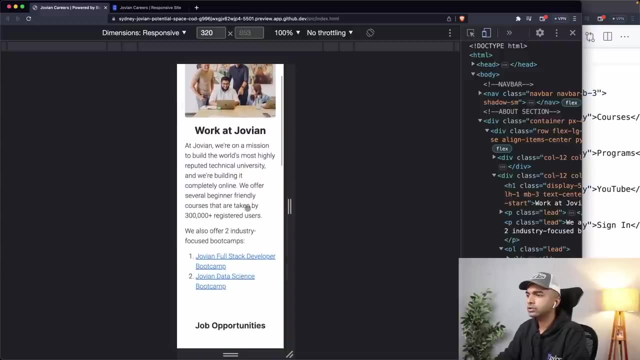 So great. This is what it looks like on. let's just go normal to the basic device mode and let's see things from scratch. So this is what it looks like on mobile. There is, There's this nice drop, There's this nice menu here we have, and then we have work at Jovian and maybe we can make. 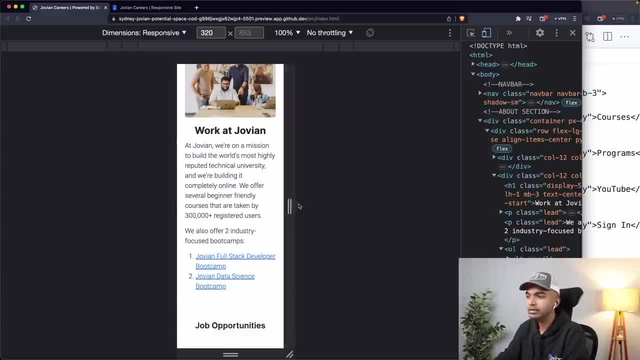 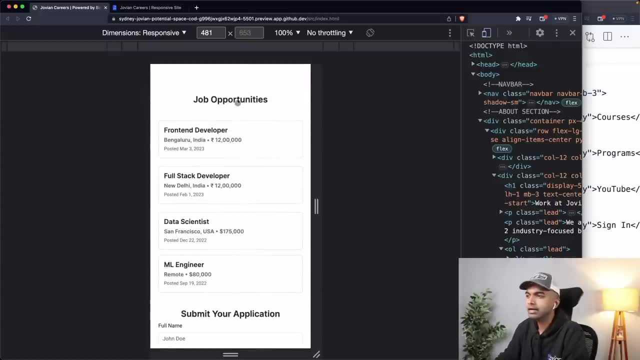 this a little bigger on. maybe we can make this a little smaller on mobile. I let you maybe explore that as an exercise. then we have job opportunities. Maybe we can make this heading a little bigger. I let you experiment with that as well. 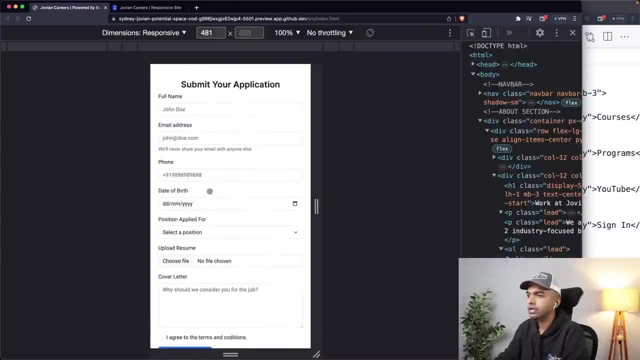 Then we have submit your application. Then we have the form here: full name, email address, phone, date of birth, et cetera. upload resume, cover letter, agree to conditions, submit application And then we have a footer. 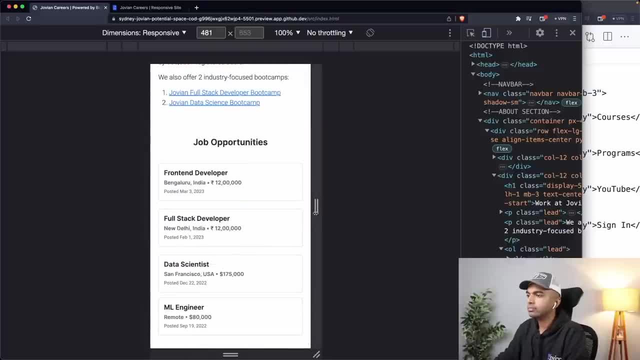 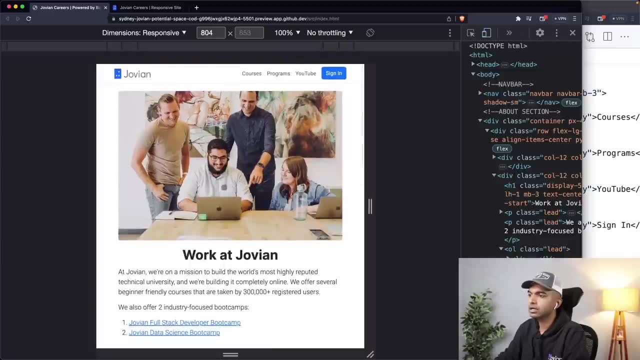 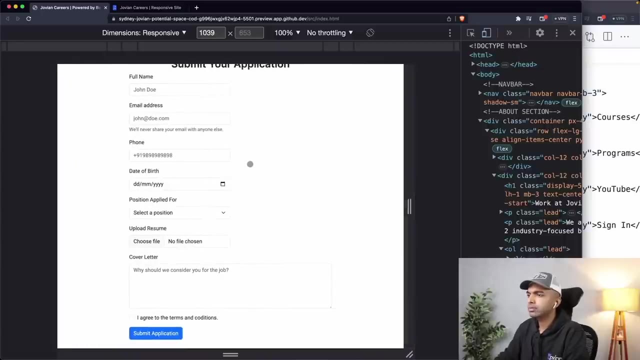 Okay, As soon as we get into the MD layout, the cards disappear and this appears, the table appears, but we still have this vertical layout for the hero section And the form seems to take up the full weight When we get to LG. then this now becomes horizontal as well. 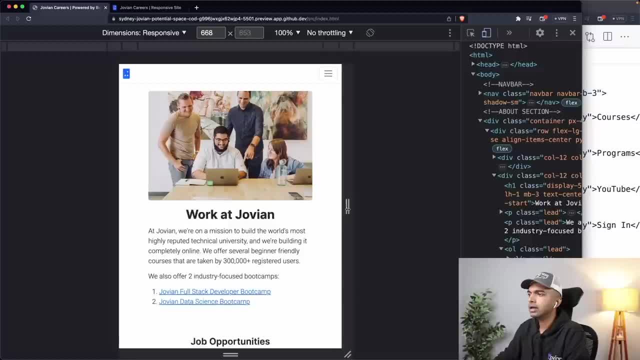 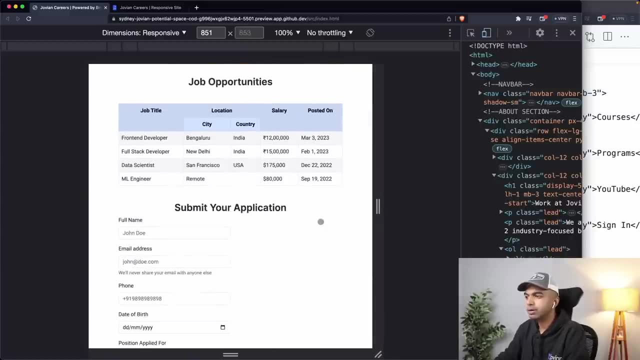 And these open up as well. You can see that on empty to these open up and on SM these don't. So yeah, a bunch of changes going on in each section. You can just browse through each break point and you can see that the footer also slightly. 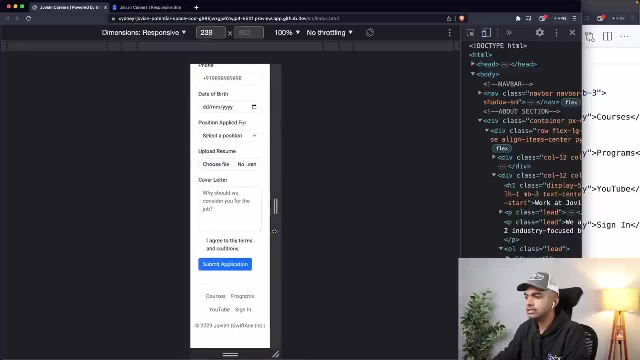 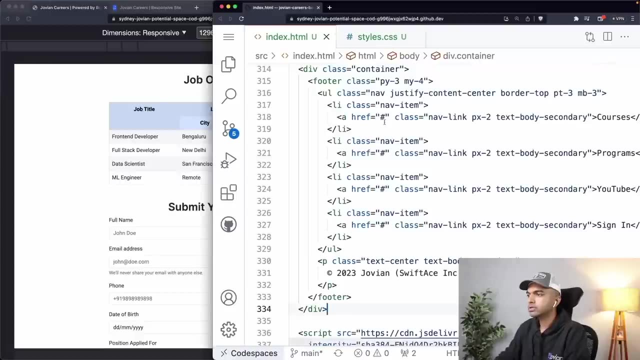 changes. You can see that the footer- here it splits into multiple lines and here then it expands into a single line, And of course, we have this nice line here as well. Okay, Yep, So I think this is looking good at this point. 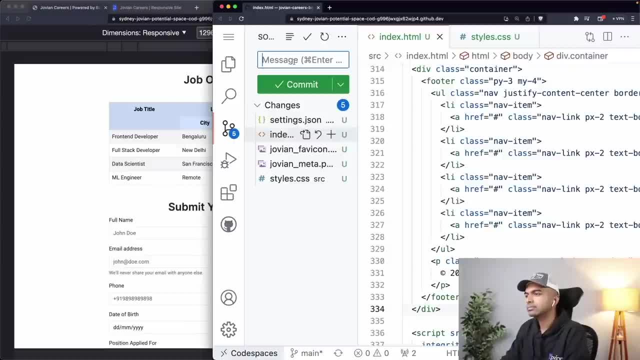 I am just going to make the changes. So I'm just going to commit this. I'm going to say added bootstrap files or sections, And I'm going to commit this. I'm going to say added bootstrap files. Okay, And I'm going to commit this and I'm going to sync it and we're ready to actually deploy. 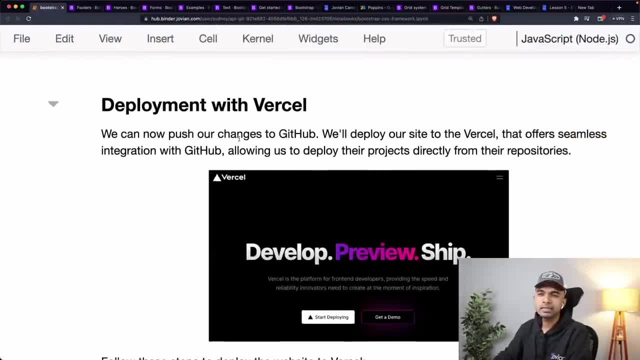 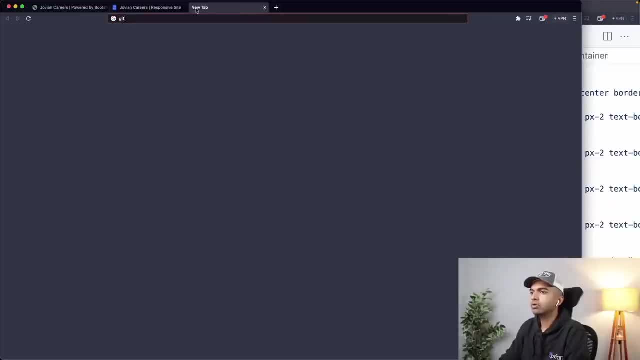 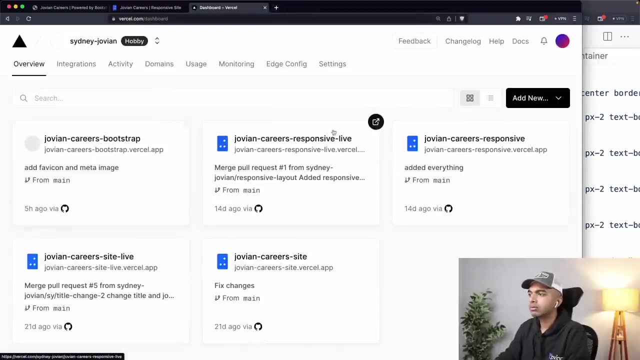 this. Okay, So this is the final step. We're going to take this repository and just deploy it on Vercel, And you know how this is. this is really really simple. So we just go to githubcom or we just go to Vercelcom and on Vercelcom, let us just 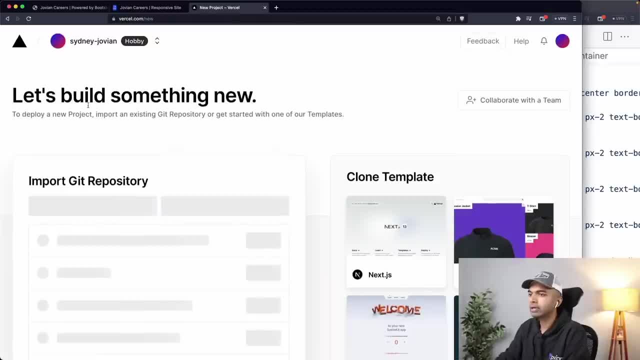 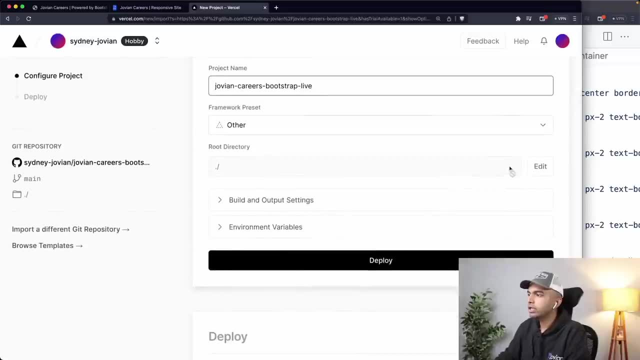 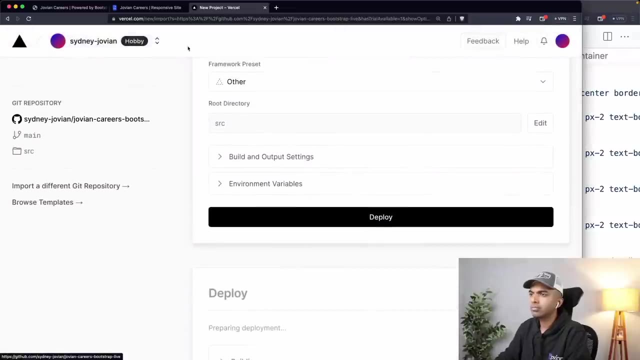 add a new repository and you can sign up and connect your GitHub account. So let's add the repository Jovian careers bootstrap live which we have created just now And we are going to. the root directory is the SRC directory, So I'm going to select the SRC directory and I am on the main branch and I can click deploy. 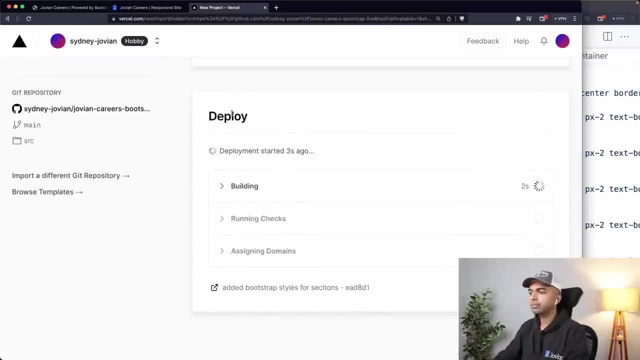 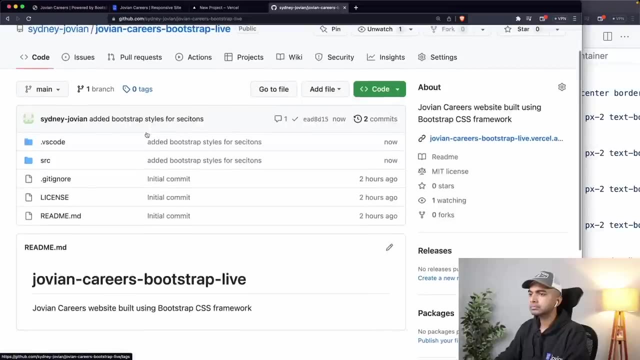 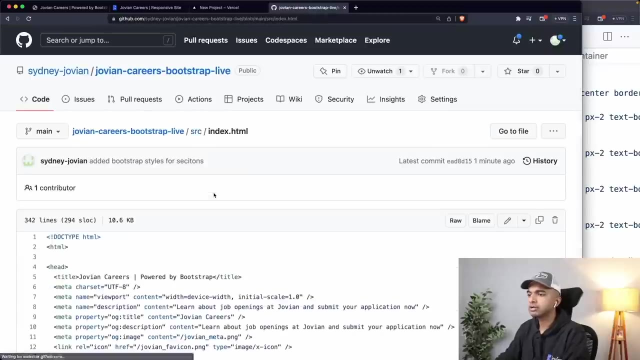 And now it is going to take the code that I've just pushed to the Git repository. You can see that we can actually see what the change that was just made. Yep, So we just added the bootstrap styles for sections And in the SRC folder we have this indexhtml file which contains bootstrap. 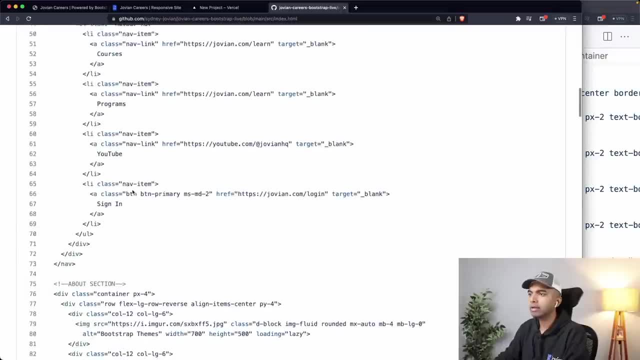 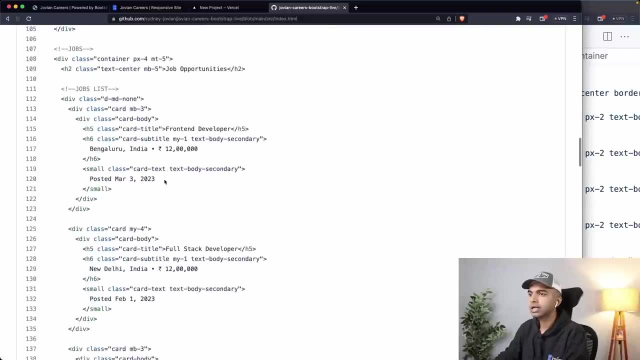 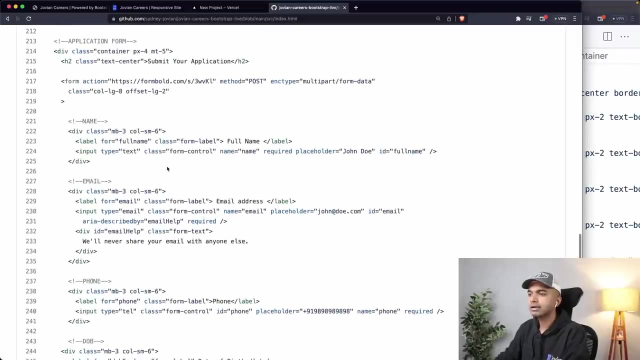 It contains the navbar. It contains the logo toggle button, the collapse section, It contains the about section with the hero image and it contains a description and links to the bootcamps. It contains the list of jobs- So this is a normal list of cards- and it contains a table with bootstrap styles and it contains 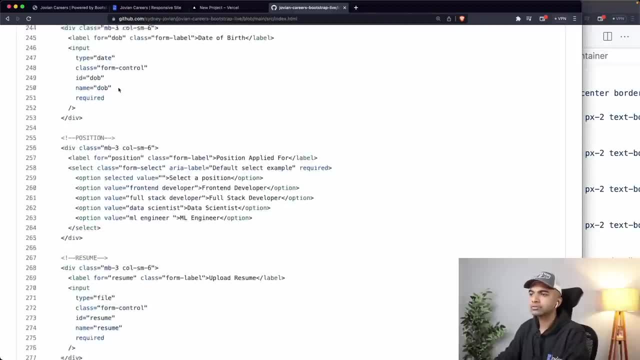 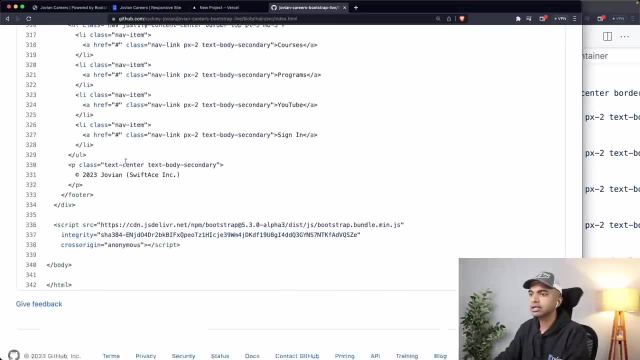 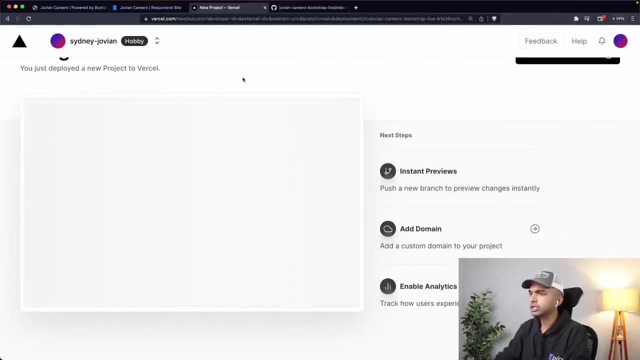 an application form and it contains the application form. contains various types of inputs, contains a position resume, cover letter, et cetera. contains terms, contains a submit button, contains a footer. and that has just been deployed. So in just under two or three minutes, we've deployed our project to Vercel. 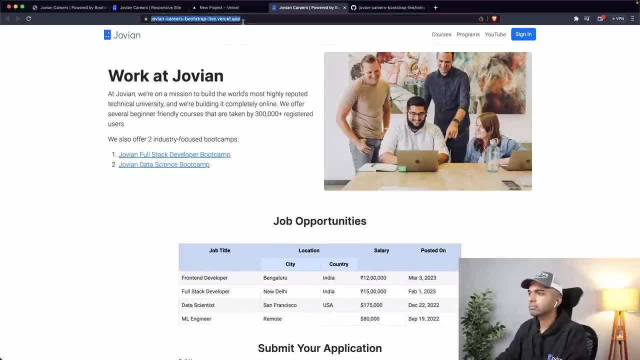 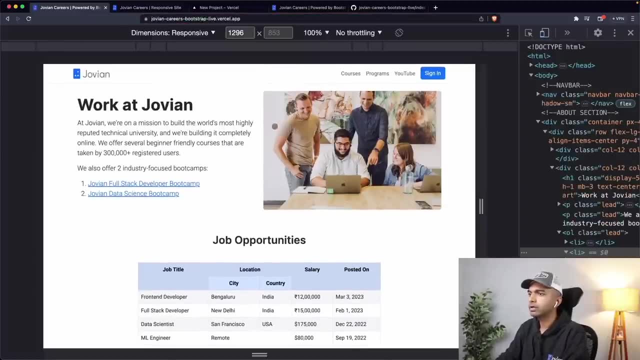 Now we can open it up and check it out, And of course it is a fully responsive website, so we can actually just open it up here in our device mode view and we can check out the links. The links seem to be working fine. 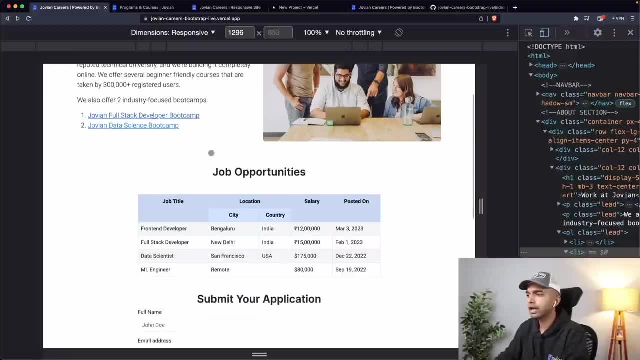 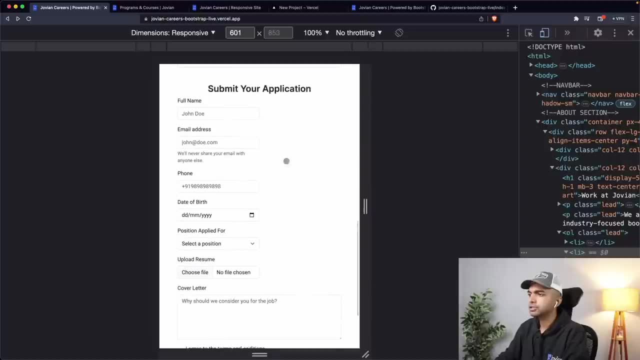 Okay, Okay, It seems to be updated to open in a new tab. We can check out that job opportunities show up properly. All right, This is good. Submit your application. This looks fine too, And let's just try filling out the application as well. 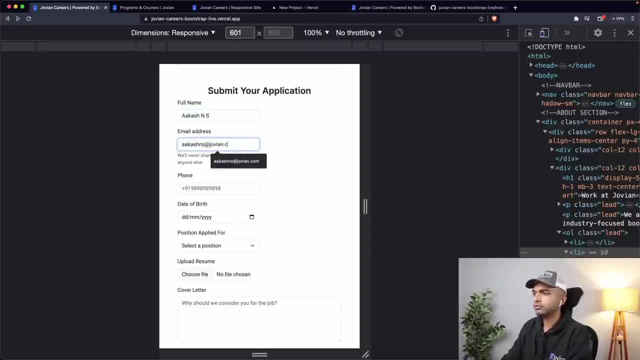 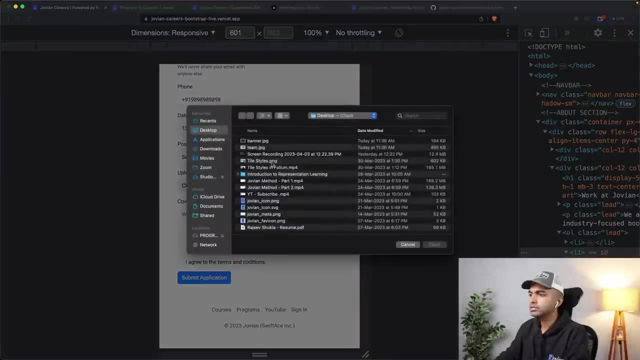 Akashns, Akashns at joviancom plus nine one. okay, Let's try to hit submit and it's going to say this is a required field. So let us fill this in And let us upload a resume. 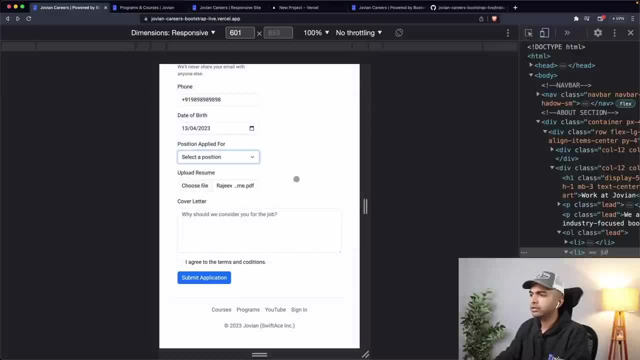 So let's grab a resume here. I'm applying for the. let's try to apply again. Okay, This is also required. So let's select that too Well. cover letter, Why? Well, I know responsive design and bootstrap. and then I agree to the terms and conditions. 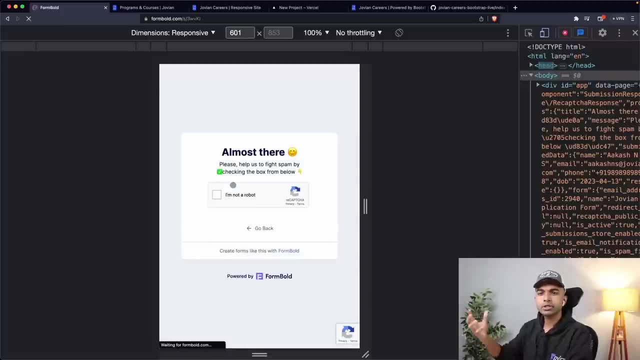 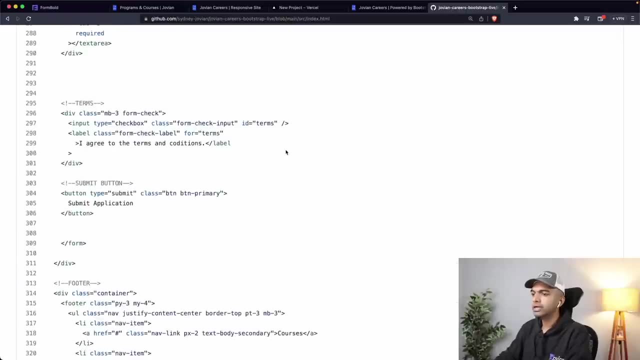 I click submit. Okay, So this is going to make a submission. Remember, we were using this third party tool called form bold. So if you check the form here, we had said the action to form bold And in a future lesson we look at how to actually handle the content. but we are simply. 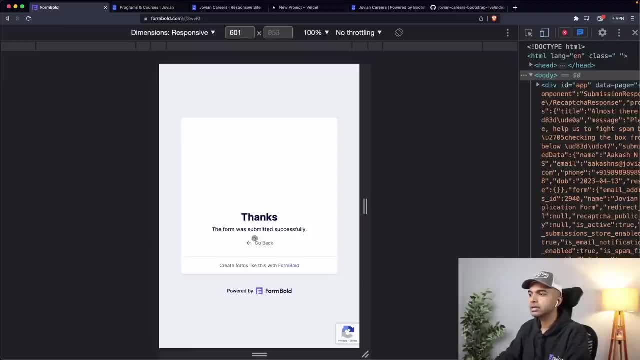 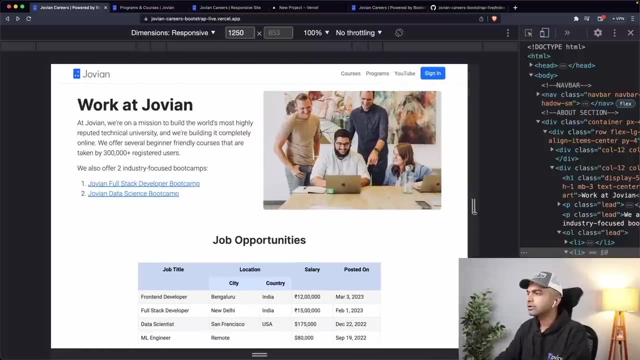 sending it to third party And that is going to then send us an email with the response. but yeah, the form has been submitted and the Jovian team will get notified. Perfect, I think this page looks pretty good now, considering where we started. 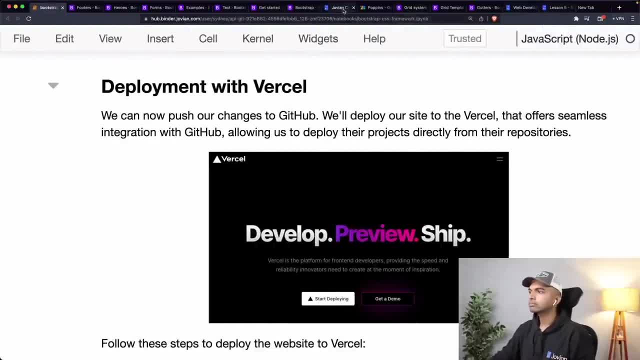 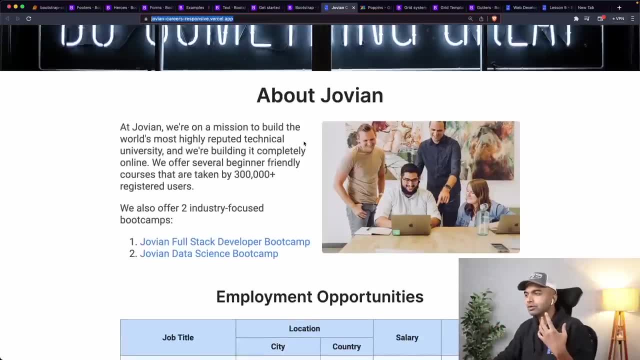 Okay, Compared to where we were the last lesson, I think this was looking good, better than what he had earlier, but it still had certain issues. You couldn't. you could tell that it's not very polished, but you couldn't tell exactly. 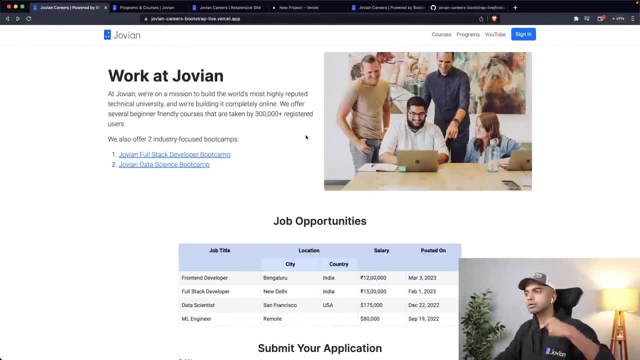 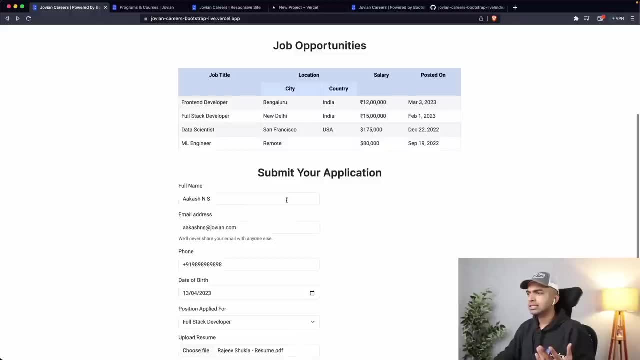 why- And that is where frameworks like bootstrap come into picture. You can use their default styles, You can use the examples that they have and you can build out these nice looking web pages. I think there's still some spacing that we can improve here. 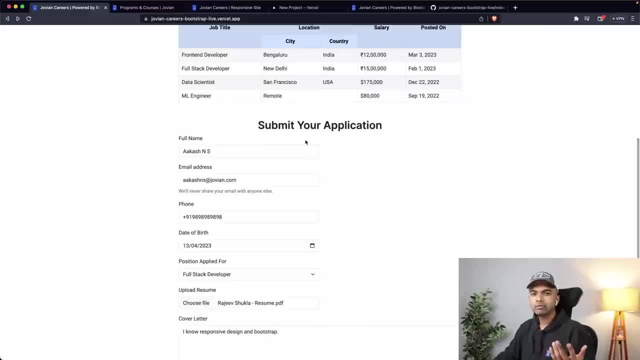 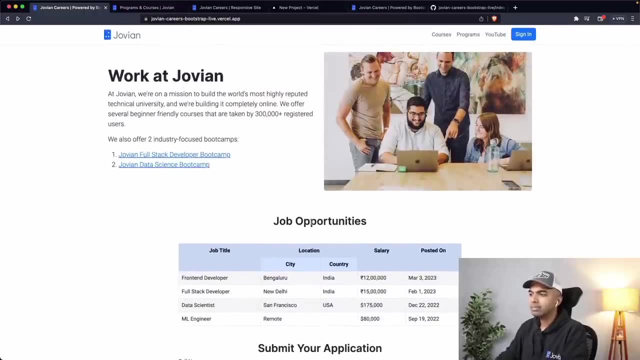 Probably. I think the spacing seems a little bit off here too. I'll let you fix that as an exercise. Maybe we can add, maybe like a subtitle or something like that, but otherwise maybe we can increase the size of this header. But otherwise I think this is looking pretty pretty good. 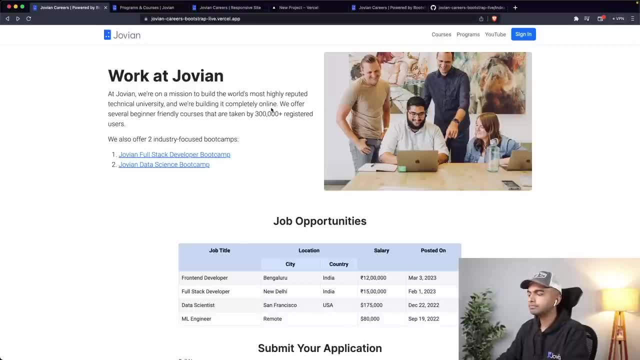 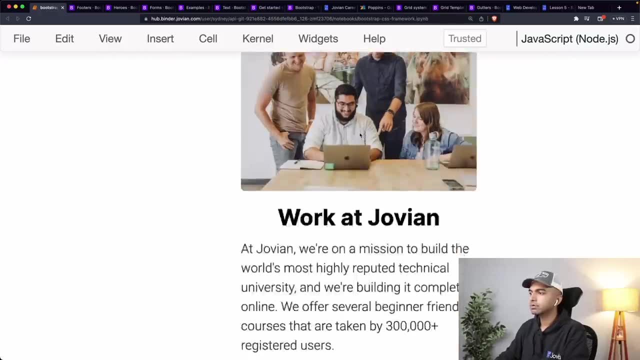 And it also has like slight interactive elements on mobile. So that's it. That is what we have ended up with. This is what the page looks like, all good, And this is what it looks like on mobile. We have these nice cards and we have this nice separation of the different elements. 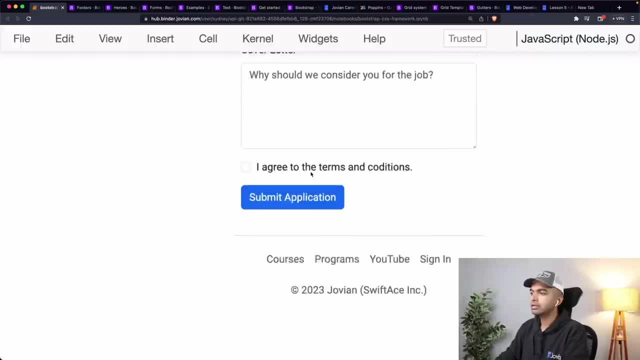 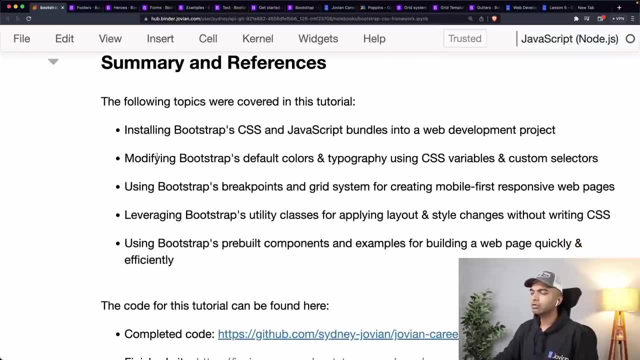 Okay, We have the different elements of the card as well. That's good. So in this tutorial, we saw how to install bootstrap CSS and JavaScript bundles into a web development project. We saw how to modify bootstrap's default colors and typography using CSS variables and custom. 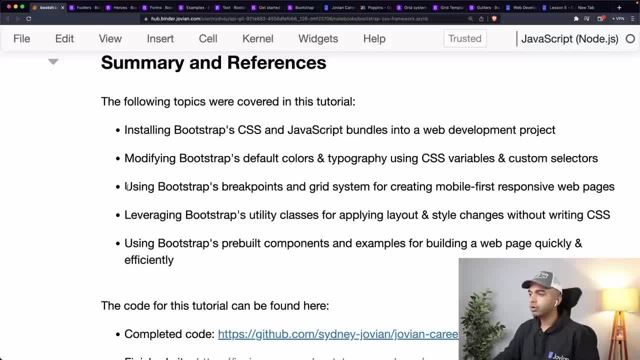 selectors. We saw how to use bootstrap's breakpoints and grid system for creating mobile first, responsive web pages. Remember, you have to first put a container, then inside it you can put a row. if you want to put columns, You can put multiple columns within the row and then you can use sizes. on a call: 12 column. 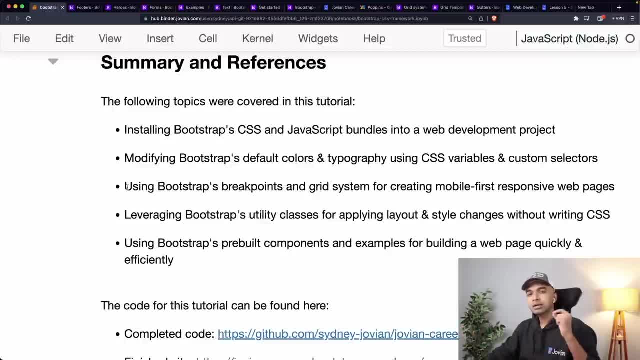 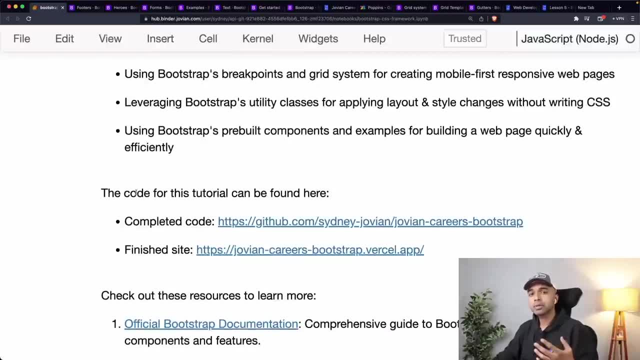 grid to arrange them. Then you can have use the breakpoints as class prefixes, And that is how you achieve all kinds of interesting layouts. And of course you have a lot of utility classes for display, for background, for text, for flex. So all those are going to be really useful as well. 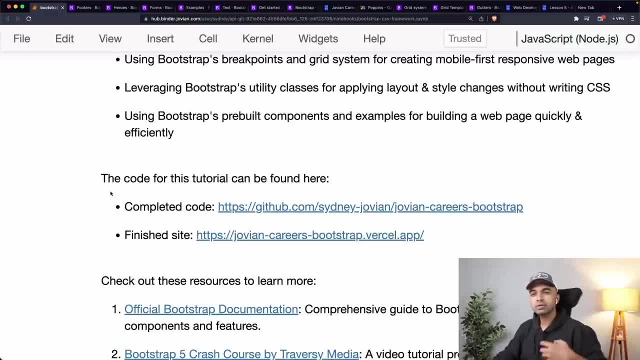 We saw how to use a bootstrap's pre-built components, So we use the navbar We built. we looked at an example hero section. We used form components, We use tables, We used an example footer And we use these for building a webpage quickly and efficiently. 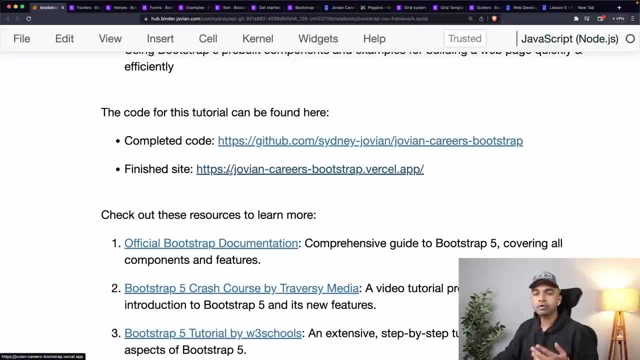 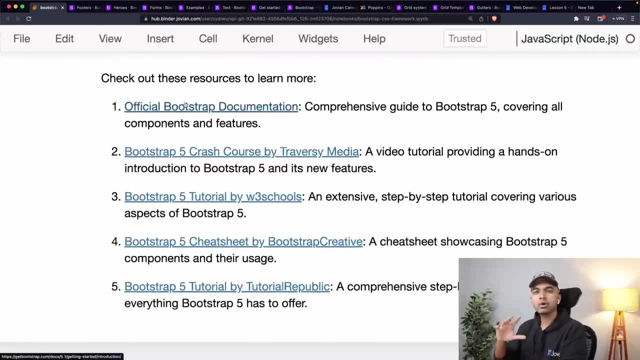 And all the code for this tutorial can be found at this link, And you can also check out the finished site, because it's deployed to Vercel automatically, And I would encourage you to check out some of these resources. The official bootstrap documentation is really the only resource that you need to work with. 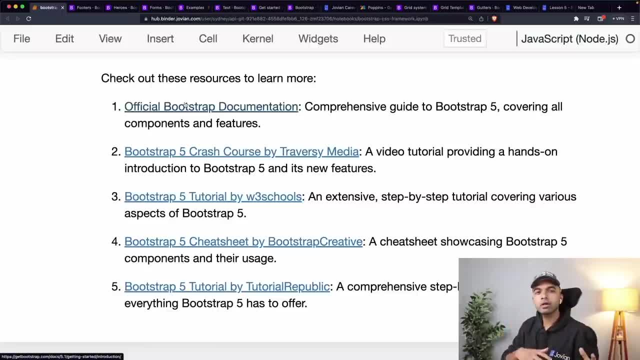 bootstrap And most of the time, what you're going to be doing is finding an example, or finding the documentation, copying or copying it over- Okay, Basically making changes to each line. always make sure that you understand what, exactly what- each class does. 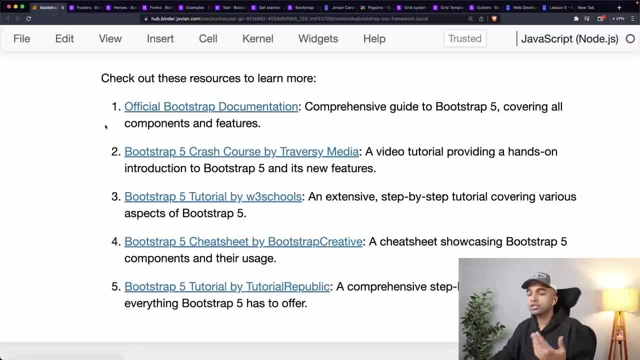 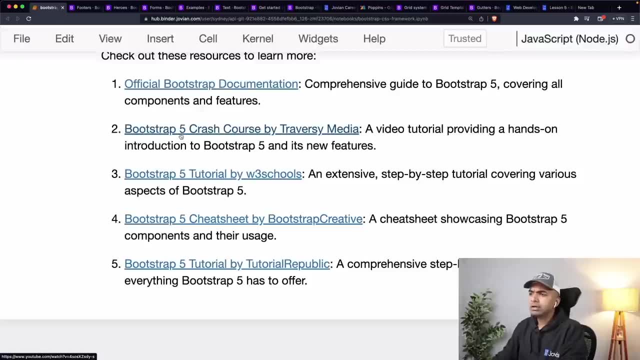 And if you're confused, try removing it. see what it does, or go into inspect element and see what it see, what explanation you can come up for it with, And then we have a bootstrap crash course You can check out, which is similar to what we did today, but a different example. 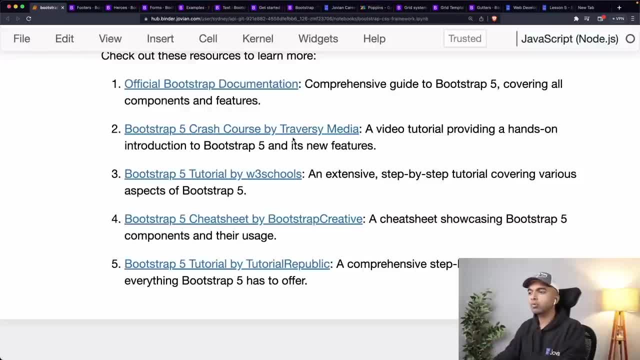 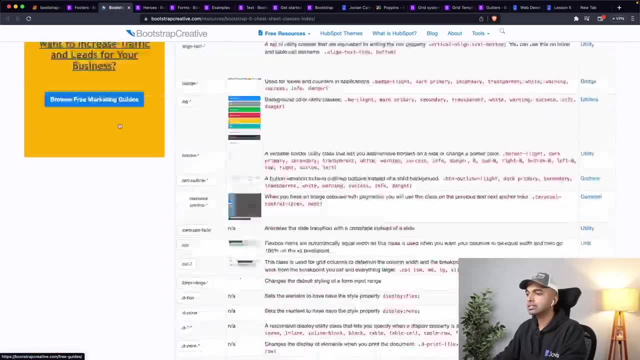 So maybe looking at a couple of different examples can help you just explore more components, become more familiar, but also a bunch of other tutorials And there's this nice cheat sheet that you can check out If you want to understand what are all the different classes that are available and what 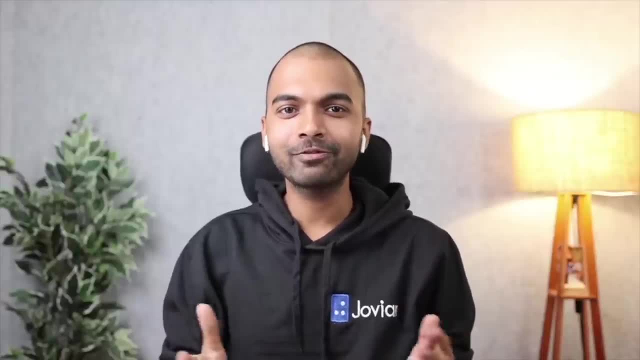 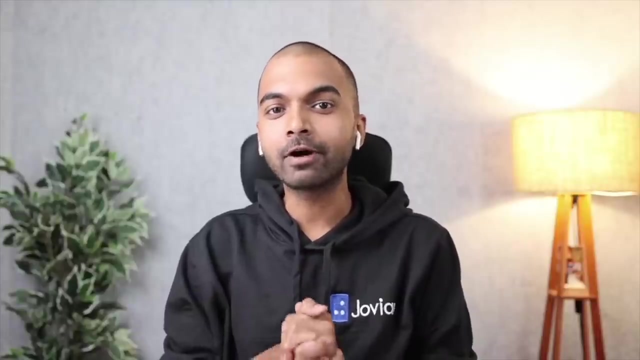 do they do? Hello and welcome to this live tutorial on building a scientific calculator from scratch using HTML, CSS and JavaScript, No frameworks required. We're going to do this all live step-by-step, and we're going to try and replicate the functionality. 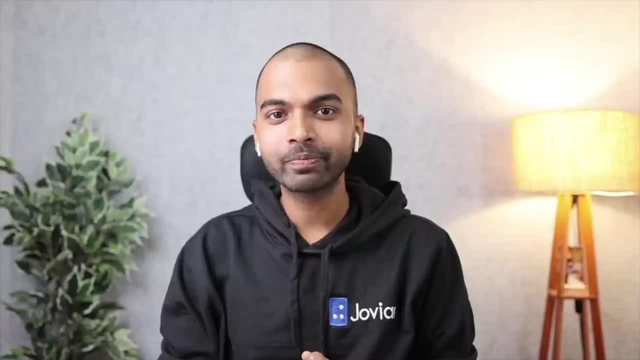 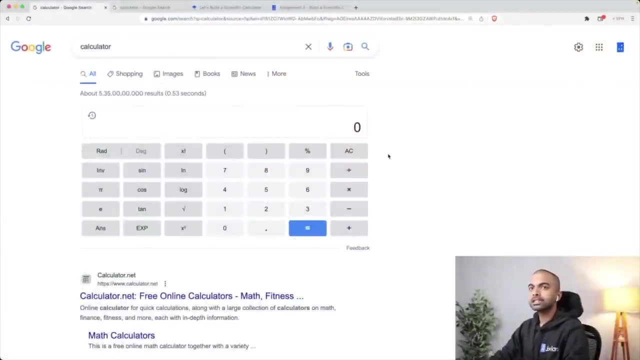 of Google's inbuilt scientific calculator and stay till the end, because I'll also show you how you can do most of your work, simply by asking ChatGPT the right questions. So with that, let's get started Now. this is what Google's inbuilt scientific calculator looks like. 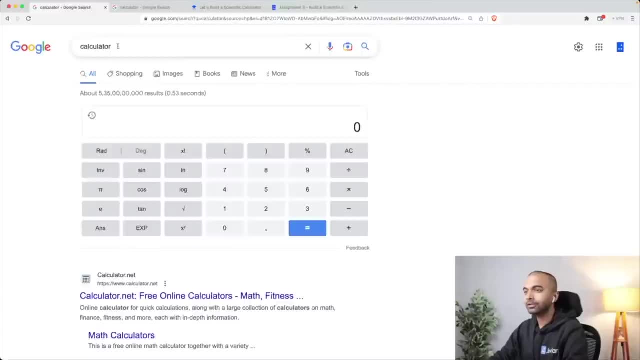 If you just head on to googlecom and search for calculator, you will be able to see this user interface and you can perform calculations here. for example, seven minus three multiplied by 69.. Okay, Okay, So you can see that this is the result: 867.079. 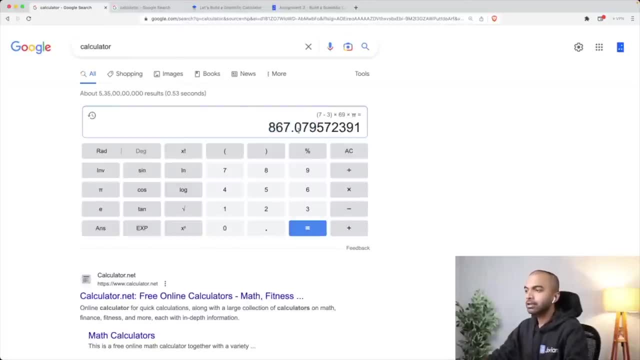 And of course, you can then use this result and build on top of it as well, But this is the basic functionality that we will try and replicate today. You can see that there are a bunch of simple calculator buttons here, and then there are a bunch of more complex scientific calculator calculation buttons that are also included. 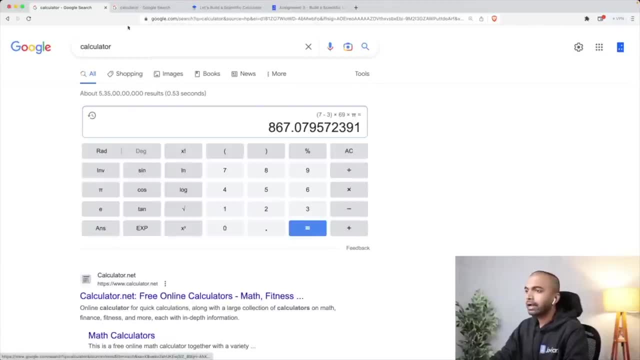 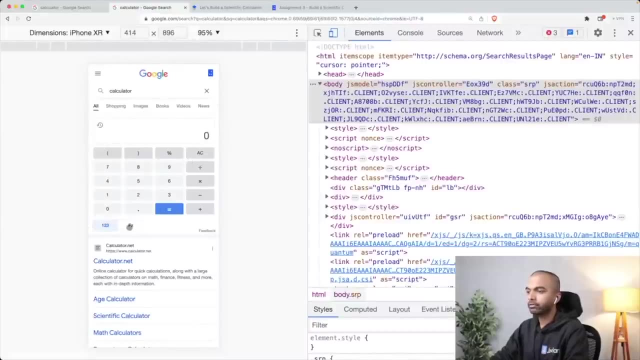 here. So let's see how many of these we can actually implement. And this is what the calculator looks like on mobile. So here is the user interface on mobile And here all the functions are under this other tab, FX. So we'll try and replicate maybe some of this functionality as well. 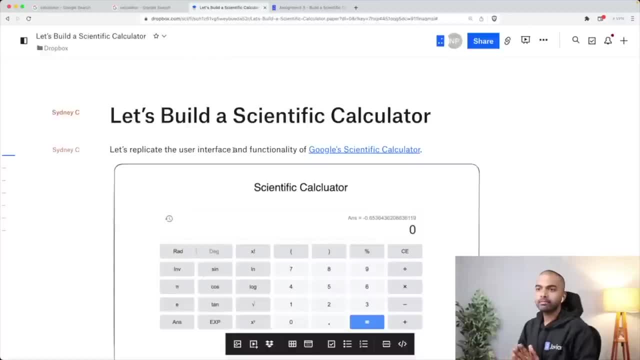 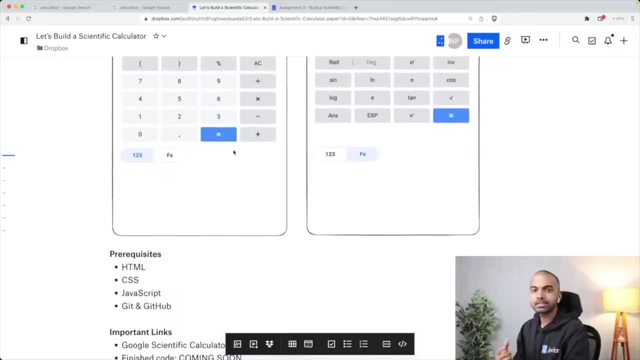 And we are going to do this step by step using just basic HTML, CSS and JavaScript. So all the steps that we're going to follow are listed here in this doc, which is linked from the description, So you can follow along if you'd like. 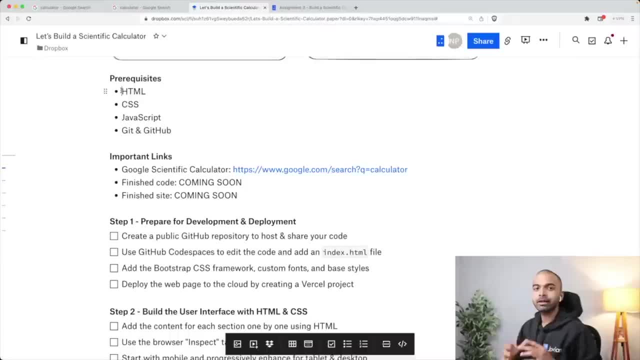 Now there are some prerequisites here. You need to know a little bit of HTML, a little bit of CSS, A little bit of JavaScript and a little bit of Git and GitHub. Now don't worry if you're not an expert in any of these, because we are going to cover. 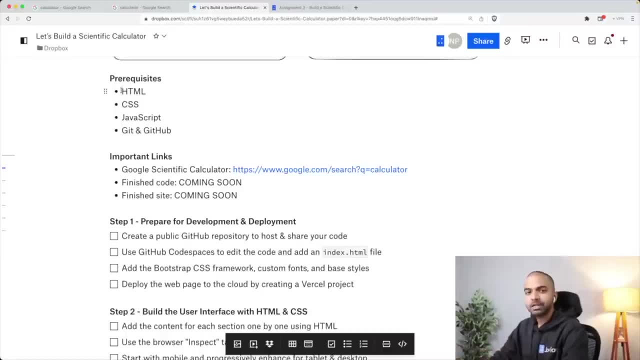 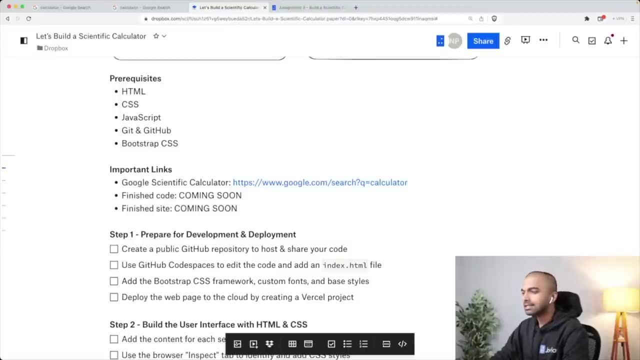 just introductory explanations about each of these as we use them. Apart from this, we will also be using the bootstrap CSS framework, And that is again something that I'll refer you to the documentation for, in case you're not already familiar with it. 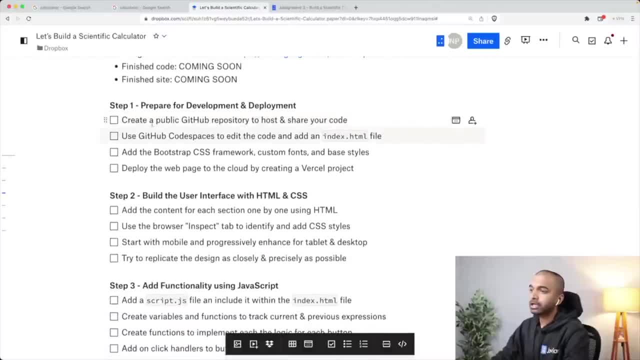 And you will be able to find the links here as well. So here are the steps you're going to take. We're going to first prepare our development. So we're going to start with the development And deployment environment. So we're going to create a public GitHub repository, launch it in GitHub code spaces to edit it. 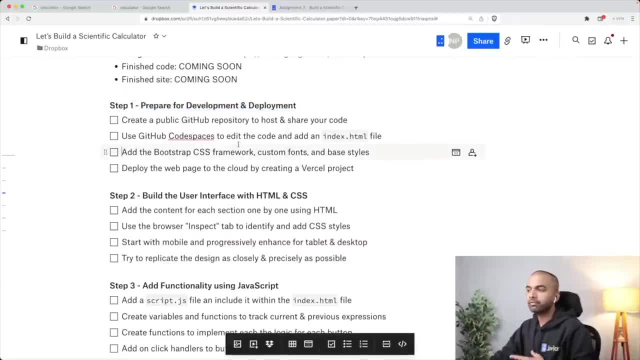 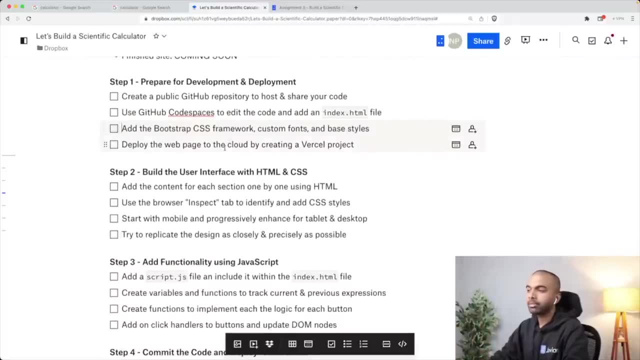 completely online. Then we're going to set up our basic bootstrap framework and also then deploy the web page to Vercel quickly so that we can test and share our implementation easily. Then we're going to build a user interface with HTML and CSS. 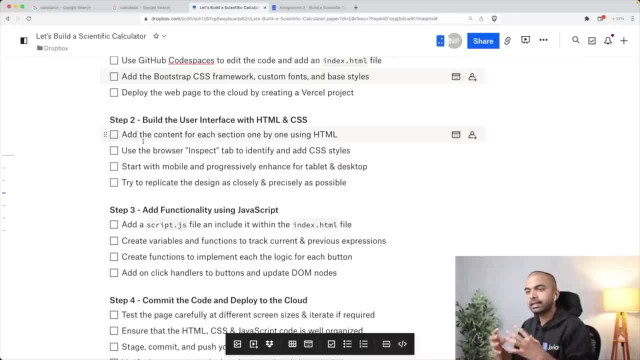 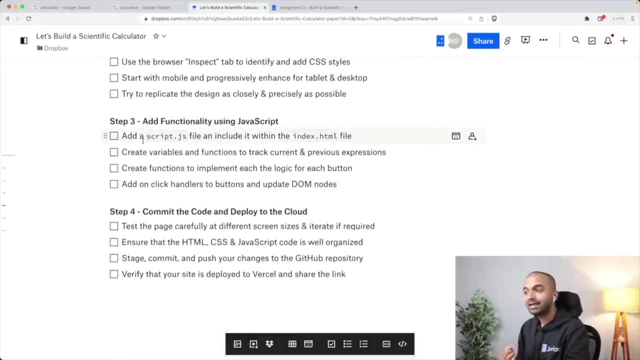 We're going to look at what the Google calculator works like And we're going to build that mobile first design and progressively enhance it for tablet and desktop. Then we're going to add some functionality using JavaScript. So this is where we're going to add a script file. we're going to create some variables. 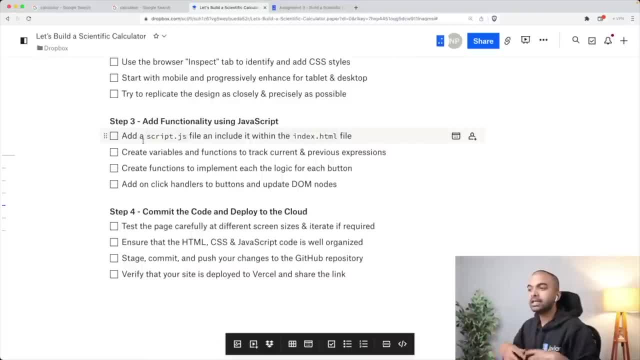 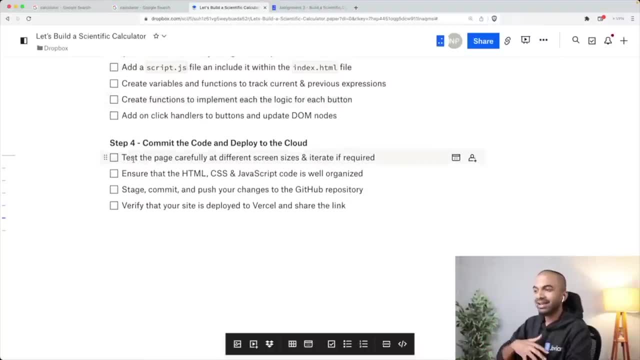 and functions to keep track of current and previous expressions. And then we're going to create functions to implement the logic for each button and add some click handlers as well. Finally, we are going to test the page carefully on different screen sizes, ensure that the 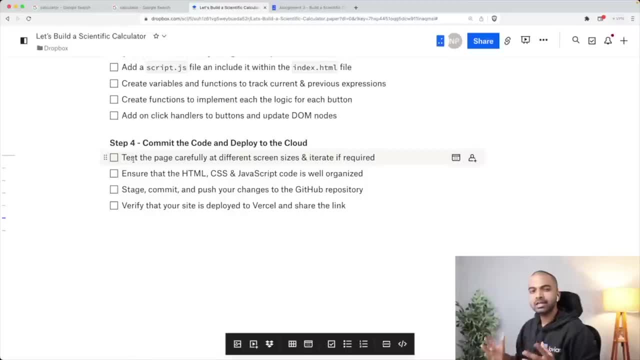 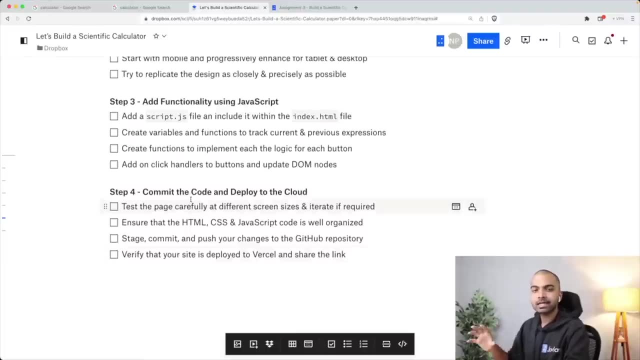 HTML, CSS and JavaScript is well organized, and then stage, commit and push the changes to GitHub and verify that the site is deployed. Now I will leave some parts of these as examples. I'm going to add a couple of things to show you how to use this tool. 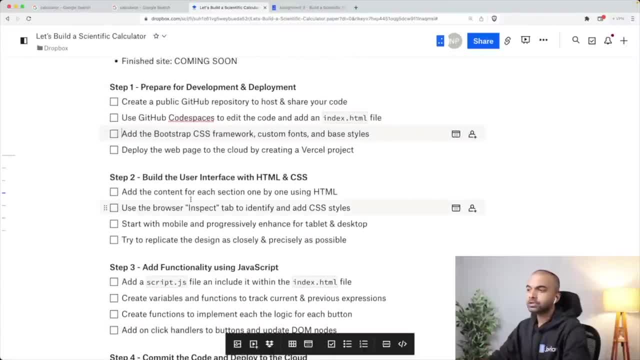 So let's get started. I am going to start with a little bit of a chat, So let's go ahead and create a chat So we'll have some chat. You can see here that we are going to use the chat, gpd and the chat. 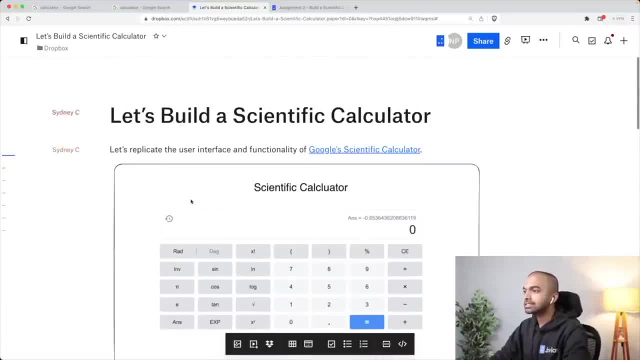 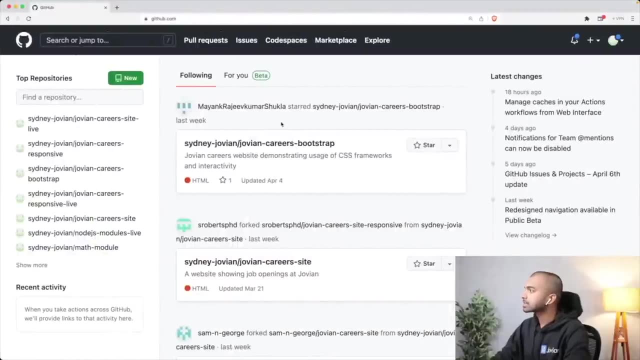 And then a couple of other things to do. So we'll see how we can build on top of what we're doing today And we'll see how far we can get in about 90 minutes or so. And then we'll also talk about how you can use chat gpd to take away maybe more than. 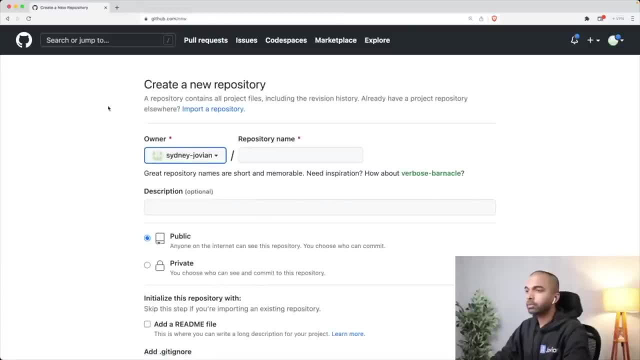 half of your work. All right, so with that, let's get started, And if you have any questions, please post them in the comments. So the first thing that I am going to do is start a new GitHub repository, and I've simply, I've simply ready to, I'm ready to put in a repository name, So let us call it. 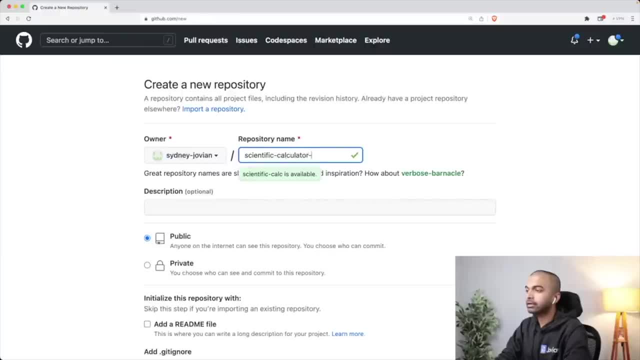 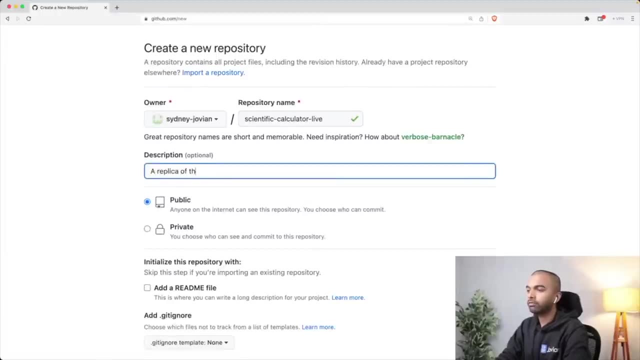 scientific calculator live, Perfect, And let's give it a description. So a replica of Google's scientific calculator built live, All right, And I'm going to make it a public repository. I'm going to make it open for everyone to use so that you can see the code. 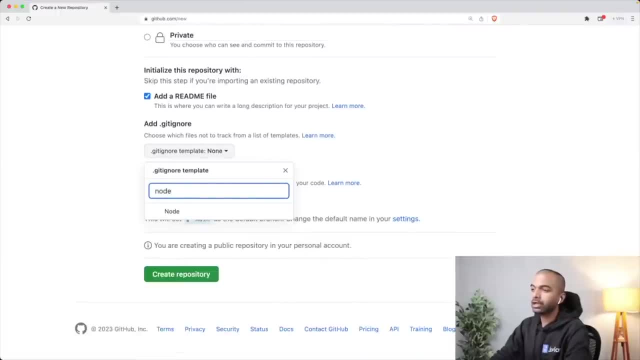 I'm going to add a readme file and I'm going to select the git ignore template node And that is going to add a bunch of git ignore settings which are going to ignore any temporary files that get created when working on a HTML or web development project. I'm going to choose the MIT. 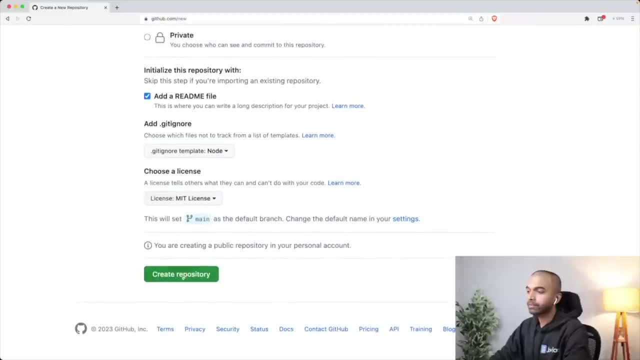 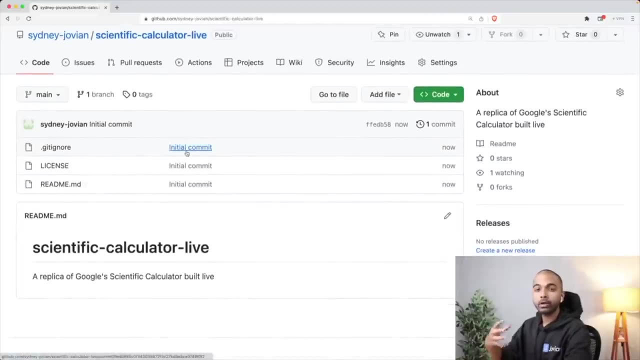 license here, because I want you to be able to build on top of this and let's click create repository And, just like that, we have our repository now created On GitHub. GitHub, of course, is the platform used by 50 million plus developers for sharing. 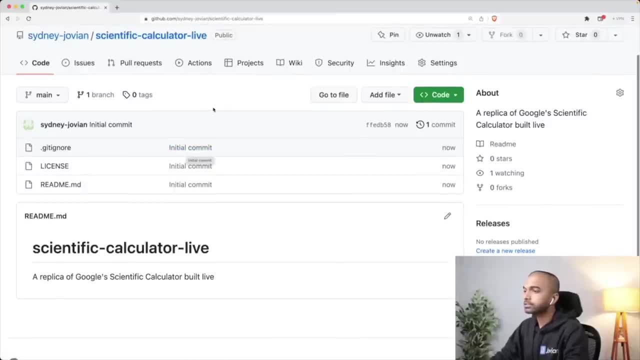 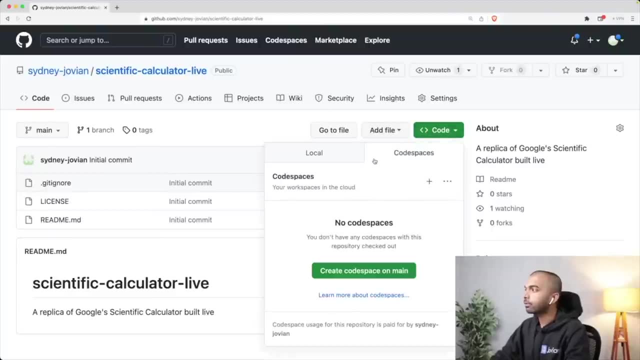 projects online. We use GitHub internally at Jovian as well And, of course, now we need a way to actually write the code, And that is where we are going to use an online coding platform called GitHub code spaces. So I'm just going to click the code button here And you can develop this. 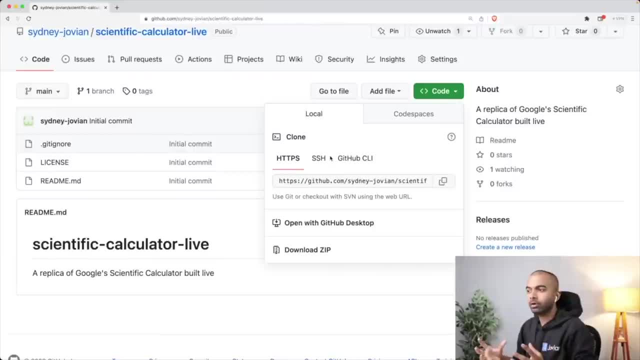 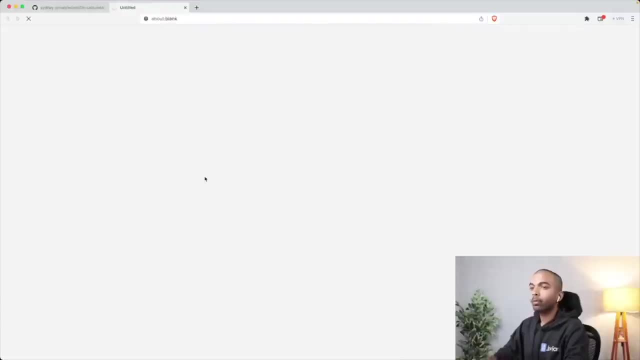 locally. you can get clone the repository and then you can run the code locally, But I'm just going to use an online coding platform. Now what that is going to do is it is going to set up a machine for me in the cloud And 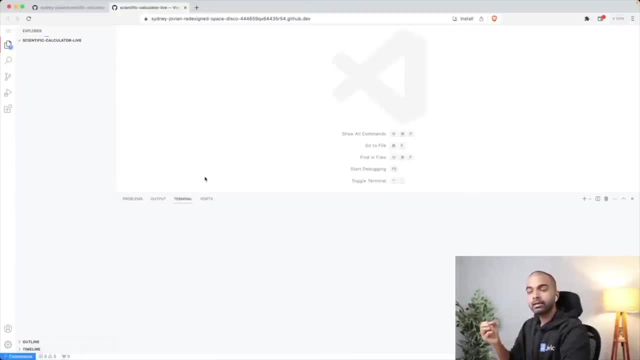 then it is going to clone the GitHub repository over there, And then it's going to give me this Visual Studio Code interface within the browser. Visual Studio Code is the editor that we use for web development and a lot of software projects, And now we can actually 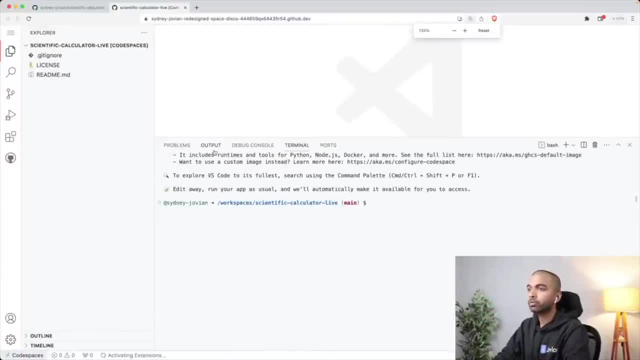 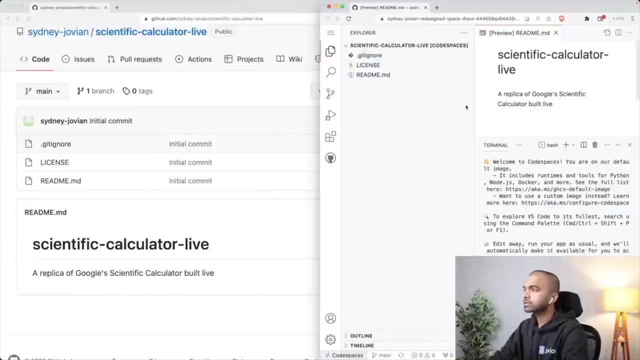 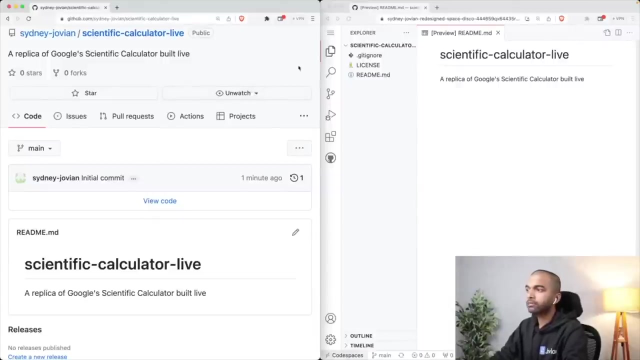 start writing our code in this Visual Studio Code browser. All right, So let me just bring this to one half of the screen So that we can be a little more organized here. I'm going to close this terminal over here And let's bring this here, And we're going to use this for just testing what. 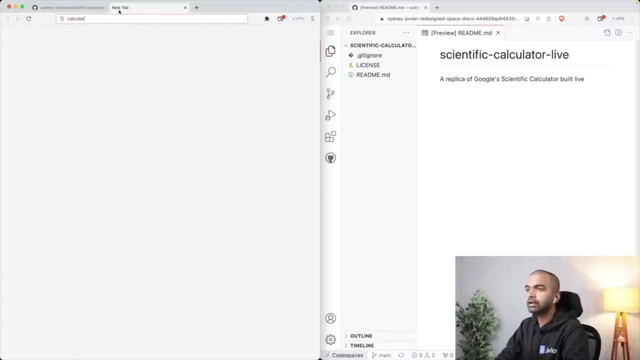 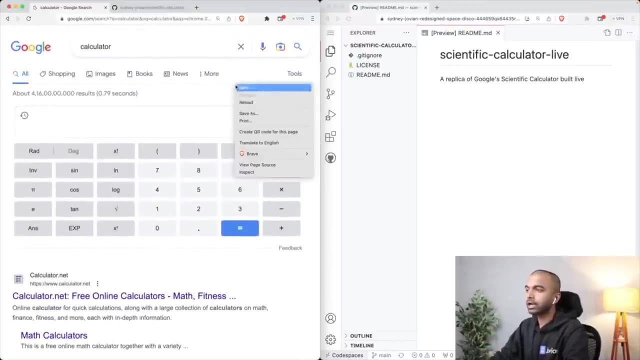 we are building. Okay, So to begin, I'm just going to go back and search calculator so that I have for reference what my calculator looks like. So this is what my calculator looks like right over here. I am just going to right click and click inspect. And generally when you inspect, 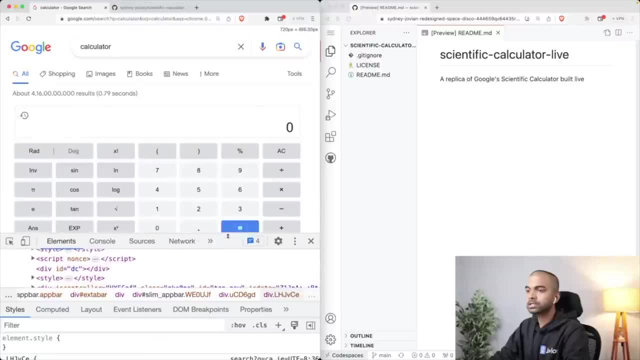 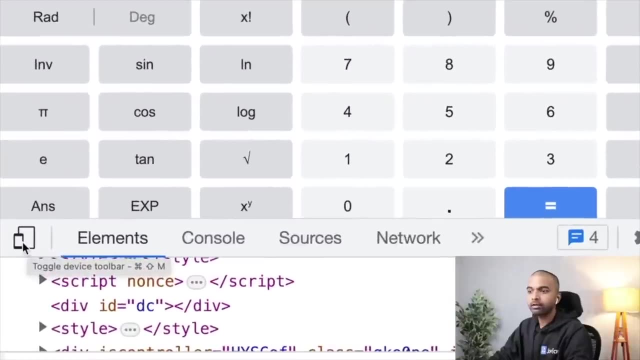 you will see a view like this. So you will see some developer tools here below your actual web page, And in the developer tools there's this button right here. This is called the device mode. So what you can do here is click this button And now you can view the. 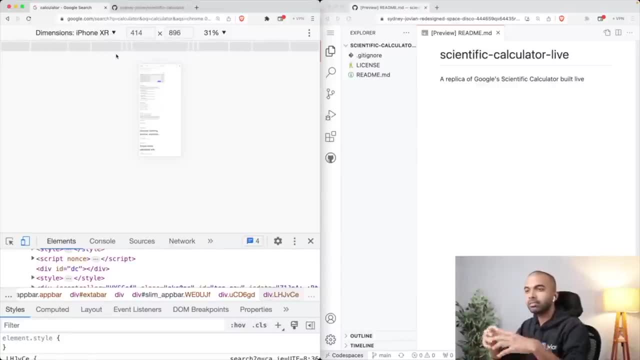 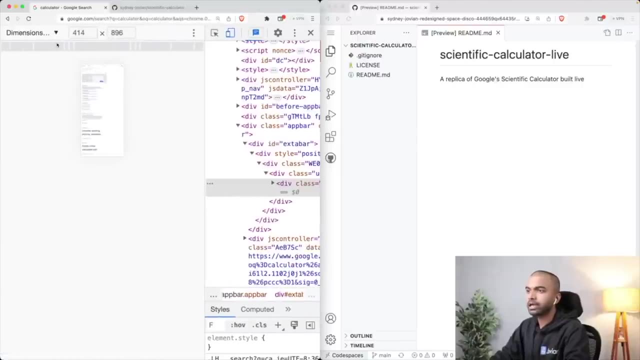 web page in a mobile device, So you can see a mobile preview of the web page, And you can also put the dock to the right side or the left side so that you can actually line it up nicely with a mobile device. So this is what. 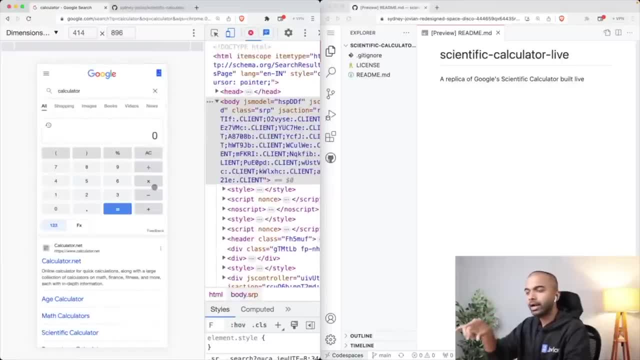 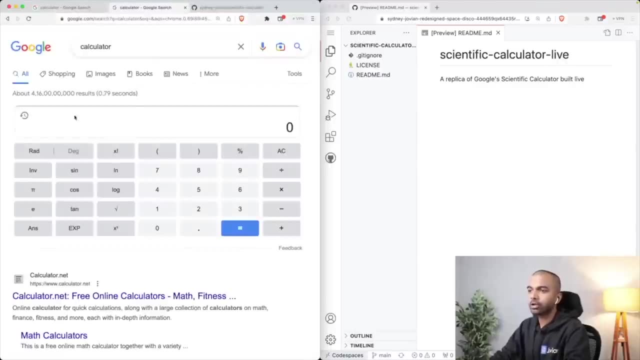 let me just reload the page. So this is what the calculator looks like on a mobile device, on googlecom, And I'm going to open up one version of it on desktop as well. So this is the normal view of the calculator And this is the mobile view of the calculator, And we're going to start. 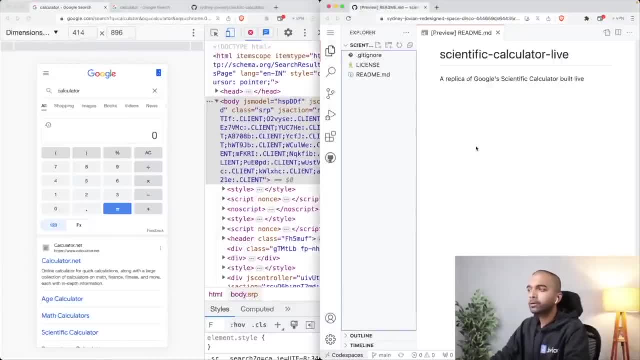 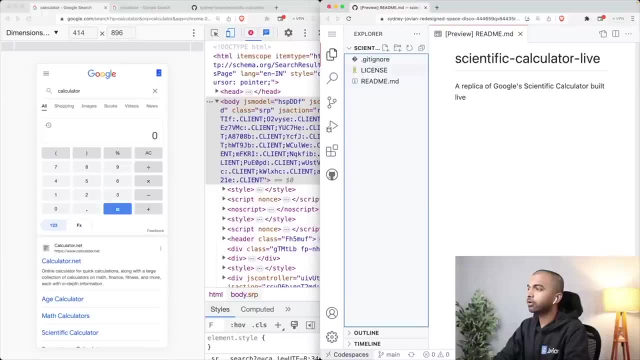 by building the mobile view of the calculator. Okay, Now to start coding. I am going to start by creating an SRC folder over here. So I'm going to just create a folder, SRC, which is where I'm going to put in all my HTML, CSS and Java. 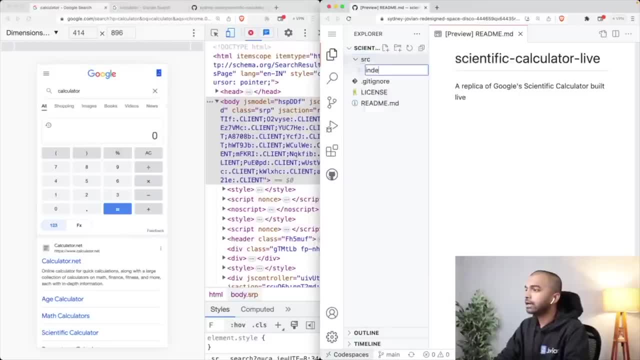 script. And now let me create a new file, indexhtml, which is going to contain all the HTML that I'm going to write. So let me just put in a doc type here, So that's something that you should always put in- let me put in the HTML tag, And in the HTML tag, let me put in a head tag And let me put in. 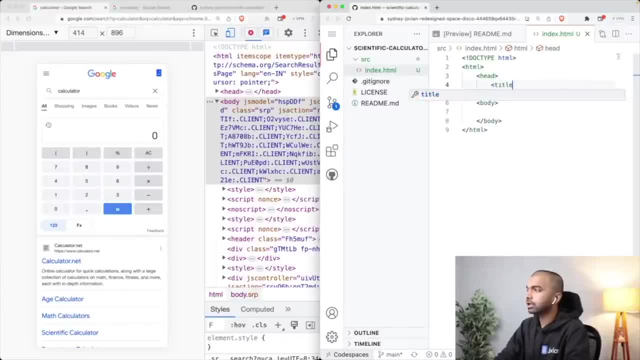 a body tag, And in the head tag let me just put in a title- scientific calculator- and in the body tag let me put in for now, just a div that says hello world, All right, So this is what we have so far. We have, let's zoom that in a bit. So we have scientific. 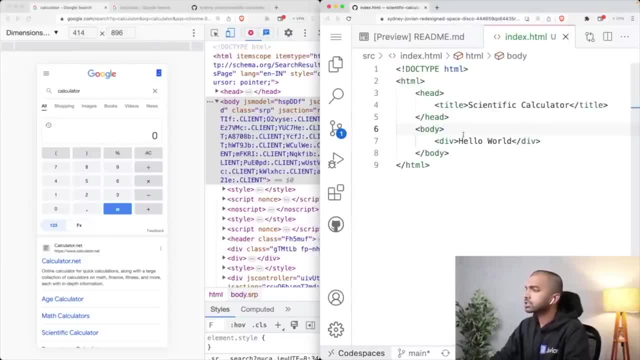 calculator. Let's get rid of this. Yeah, So we have scientific calculator. That's the title of the page. We have a body. inside the body, We have a div that says hello world. And now let us simply try and view this page. So we want to be able to preview this index. 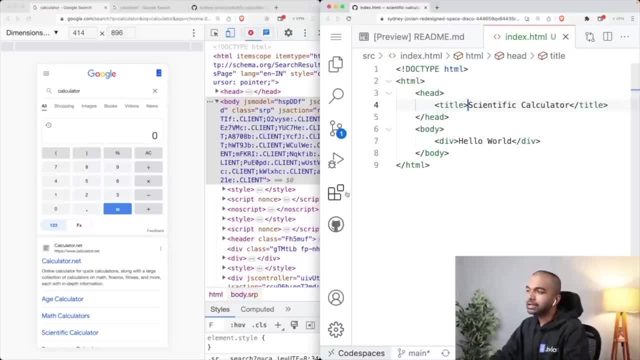 dot HTML page and to preview it we can use an extension called live server. because it's not very straightforward to preview a webpage directly from code spaces. You need a VS code extension for that. So just head into extensions and search for live server. Okay, The live. 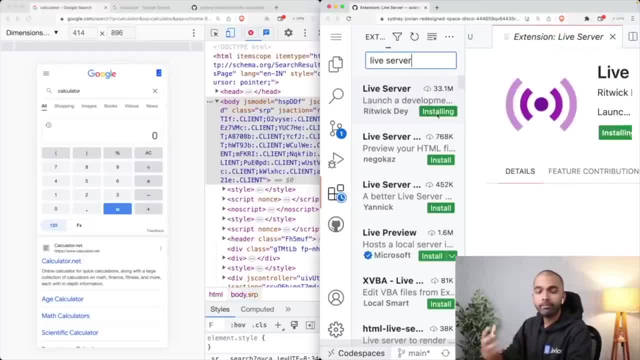 server is simply going to let us preview the webpage we are building, Okay. Okay, Within code spaces: Okay. So once this live server extension built by Ritvik day is installed, let's close this extension tab here. So extensions are found here in the menu. You can see that. 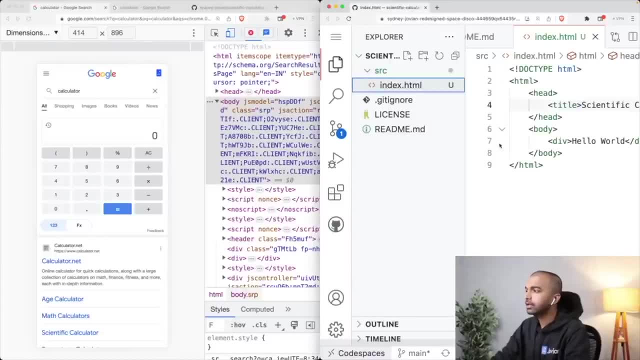 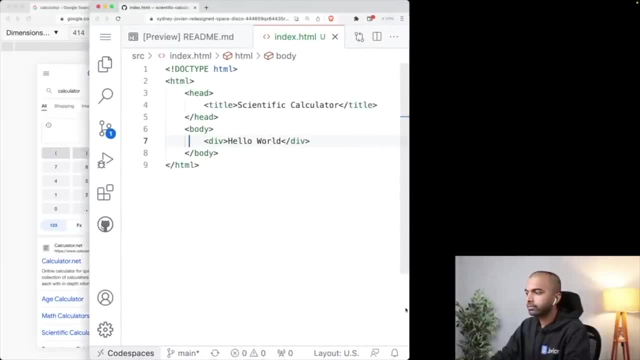 there's a menu called extension and just search for live server. install it Now. once you do that, you will see that there is a go live button. I'd have to expand this a bit. Yeah, You will see that there's a go live button at the bottom of the page and this: go live. 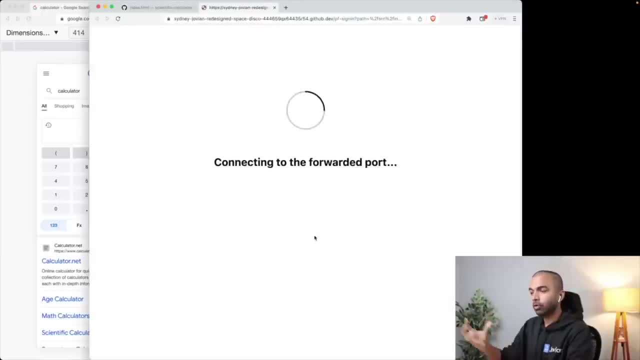 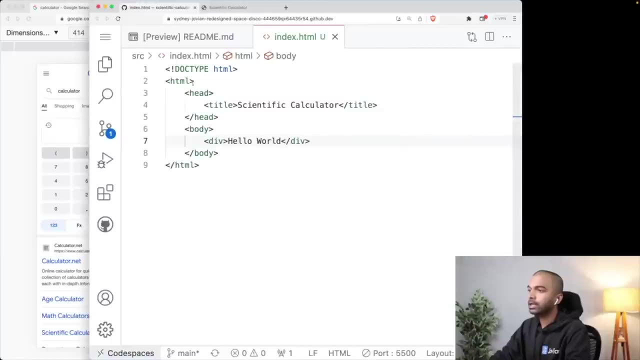 button is going to turn your code space into a server, essentially, And it's going to give you a preview of the page that you had open here. So I'd open index or HTML here And now you can see that I have this index or HTML If I zoom in a bit. 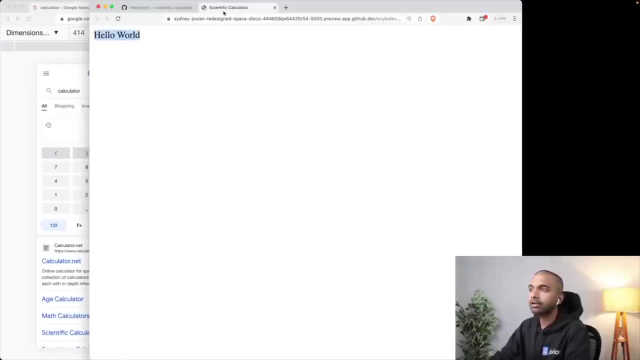 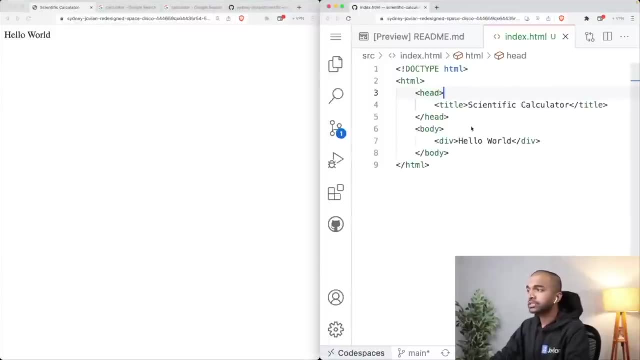 you can see the words hello world over here and you can see scientific calculator in the title. So that is how I've set up a preview of my code. Okay, So that's great. Now we have on the left we have an index or HTML file. on the right We have this hello world. 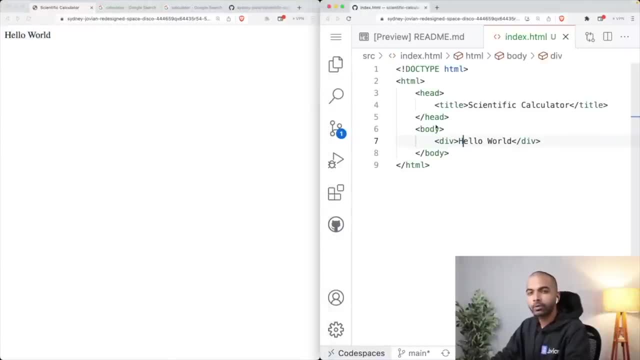 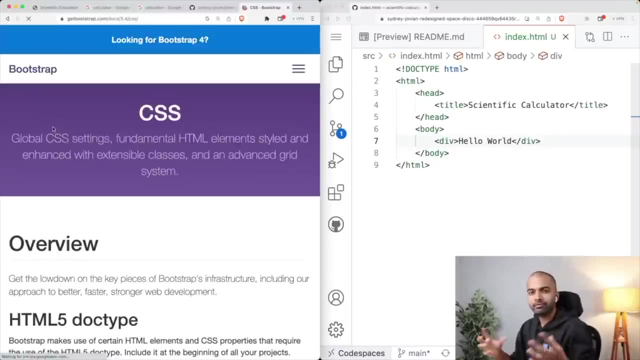 text. So that's great. Now, of course, we want to use the bootstrap CSS framework, So I'm just going to go in here and search bootstrap CSS, And bootstrap CSS makes it really easy to build very flexible layouts. It also provides a bunch of Yeah, maybe I should go for the latest version. 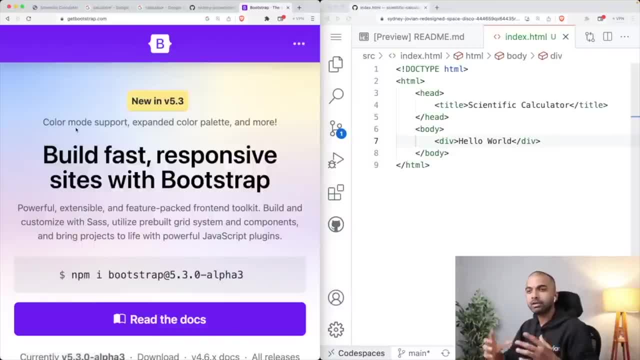 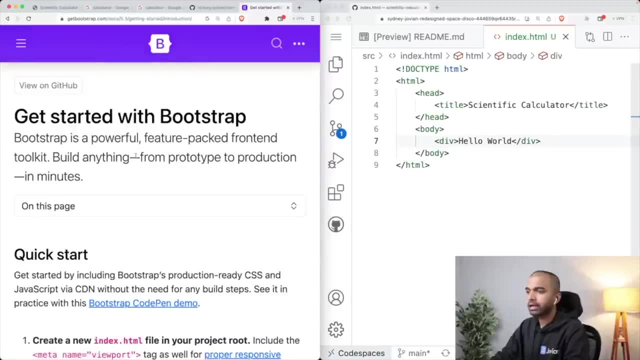 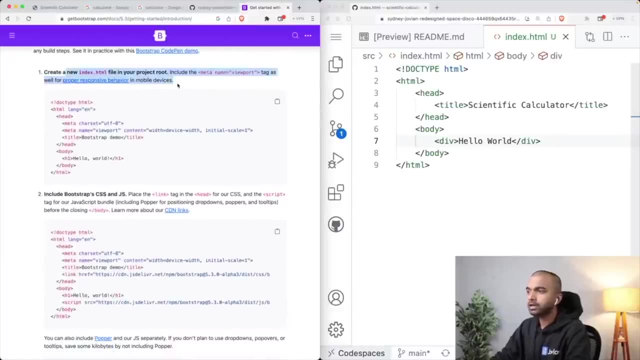 It also provides a bunch of different components that we can use, And that makes development really fast. So I am just gonna, let's see, read the docs And we want to get started with bootstrap, So let's start by. okay, it says that you need to create an indexhtml file and we need 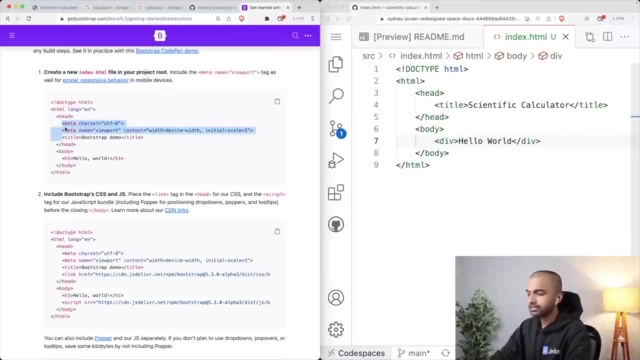 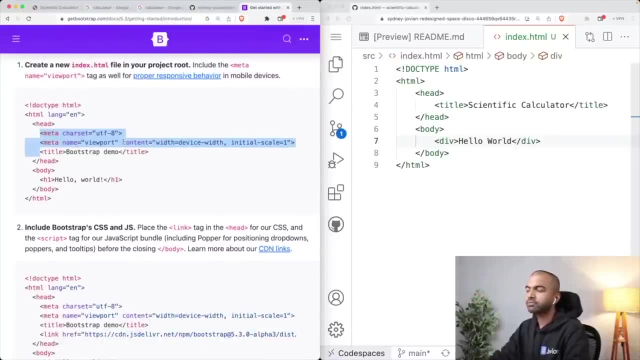 to add a couple of meta tags. So let's copy these meta tags: meta charset equals UTF eight and meta name equals viewport, So these are both required to enable proper responsive behavior on mobile devices. So I'm just going to come in and paste these meta tags in my code over here. 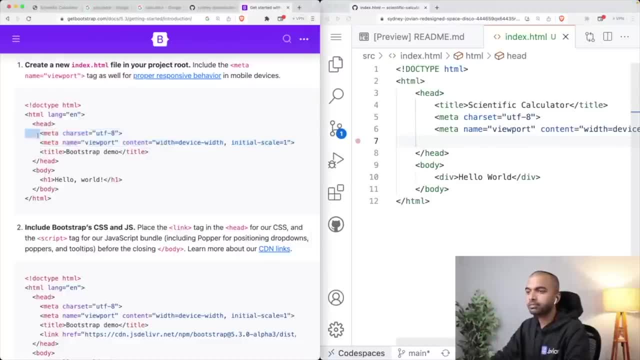 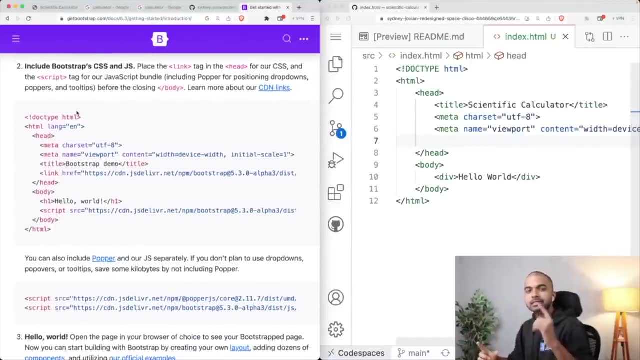 So all I've done is I've read the documentation, So read meta tags from here and pasted them here. Then the next thing I'm going to do is include bootstrap CSS and JavaScript. So bootstrap contains a CSS file which contains all the styles that it provides, And it contains a JavaScript. 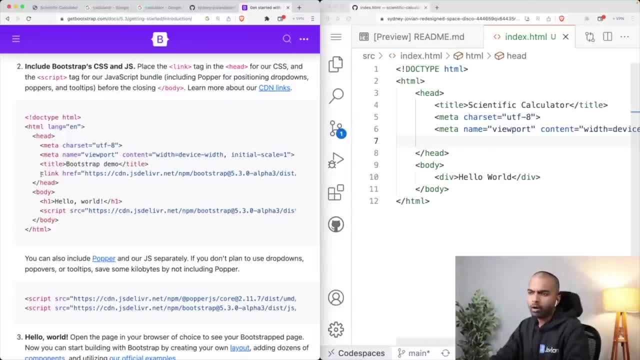 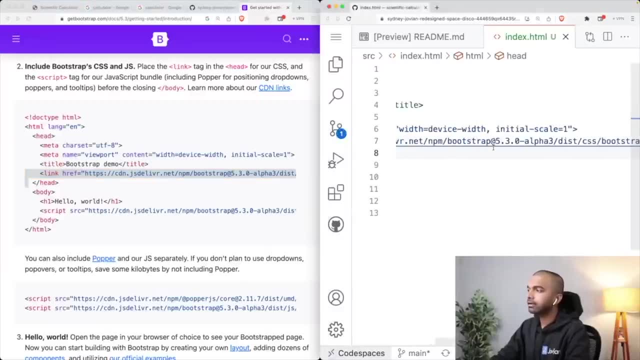 file which contains all the all the interactivity it provides with drop downs and things like that. So let's just come in and include those as well. So I'm going to include my the link tag for this bootstrap CSS file in my head tag And I'm going to include the 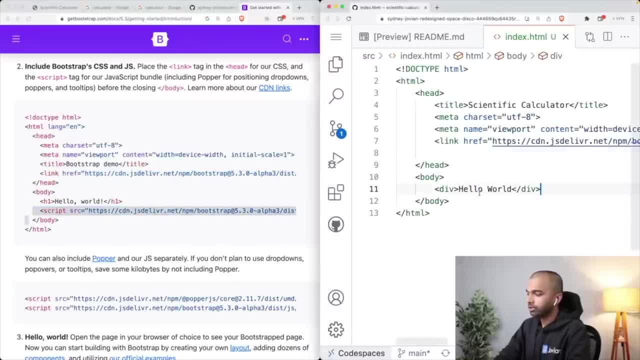 script tag over here at the bottom of the body. Okay now, if this doesn't make sense, don't worry, you can spend some time learning bootstrap, But the idea here is we're using an external framework. all it gives us is some nice things that allow us to quickly build web pages without 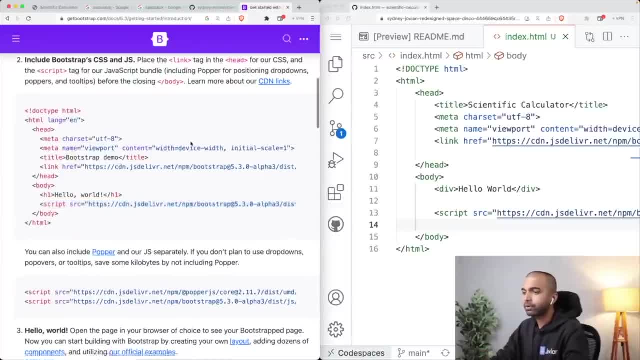 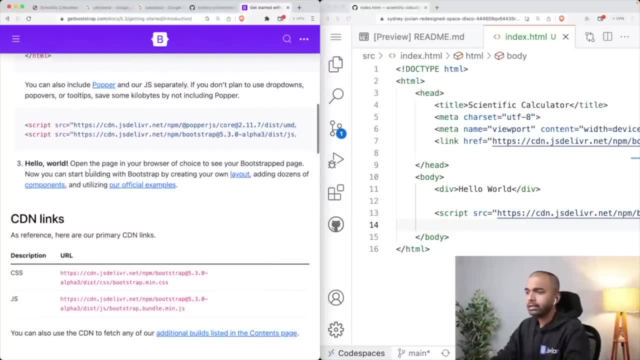 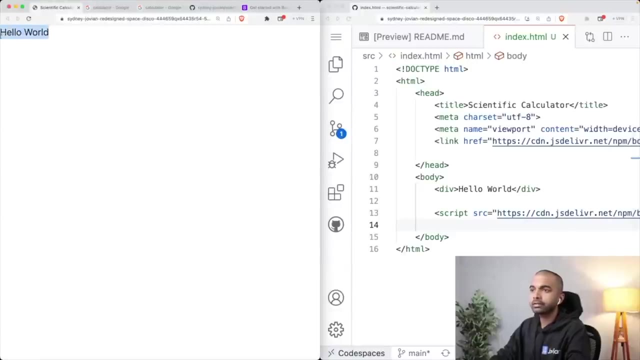 having to worry too much about writing a lot of custom CSS. Okay, Perfect. It also says you can also include popper and JS separately. Well, I'm not worried about that. So with that, I think I've added bootstrap And I should immediately be able to just see that. you can see here that the styles have immediately. 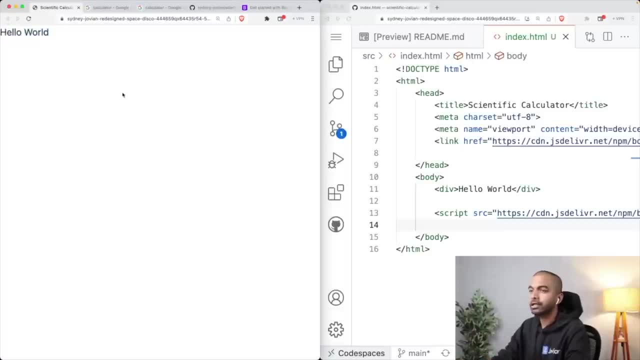 changed. I had a different font earlier and now I have a slightly different font, So that's great. Now we've added bootstrap as well, And at this point I my web page is looking pretty good And I think I'm ready to start building my scientific calculator. But let me also save the work I've 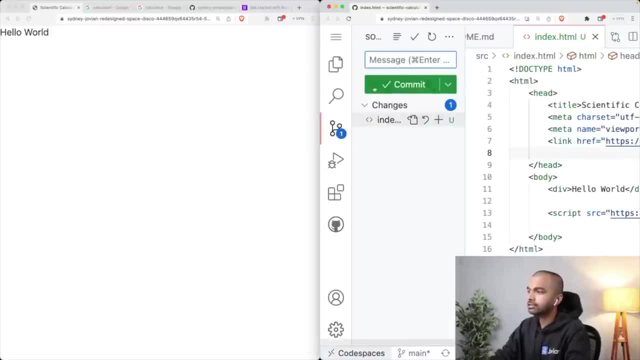 done And the way I'm going to save it is simply by adding So going into the git tab in Visual Studio code and adding a comp, adding a commit message to perform a git commit. So I'm just going to say here: 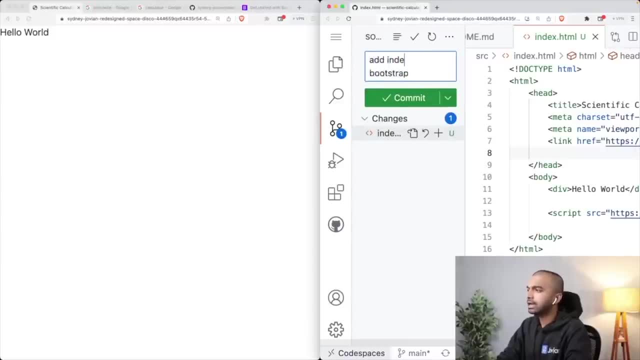 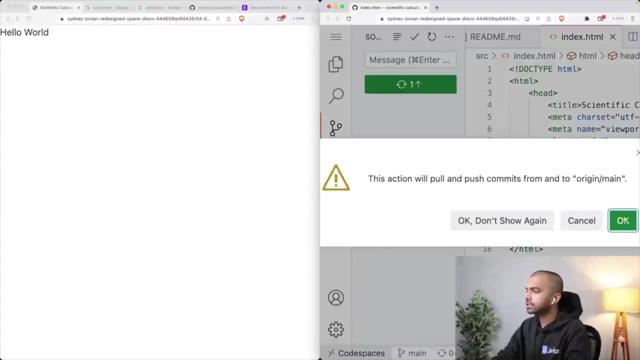 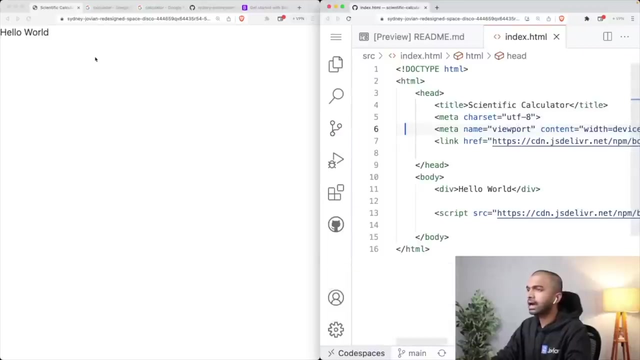 add bootstrap. Let's see add index dot HTML and bootstrap. And I'm just going to click commit And it's going to ask me a few things And it's going to just commit those changes And that's it. And now this is going to get pushed. So you press the sync button And that is going to now push that. 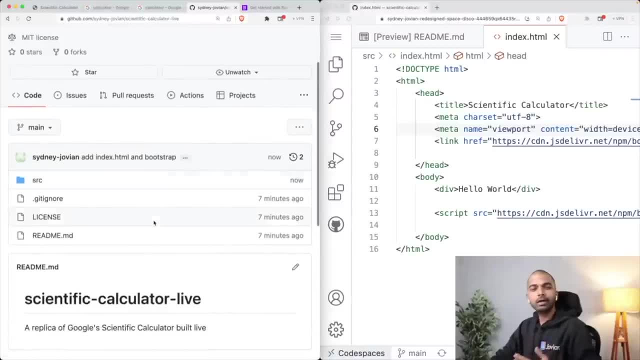 code back to the repository. Okay, so that, of course, is the git workflow. you open up the code either locally on your computer or on a GitHub code space, then you make some changes and you test them out using a live server or some kind of a server, And then you commit and push. 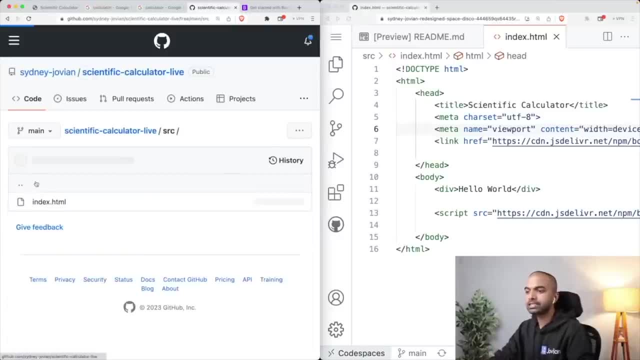 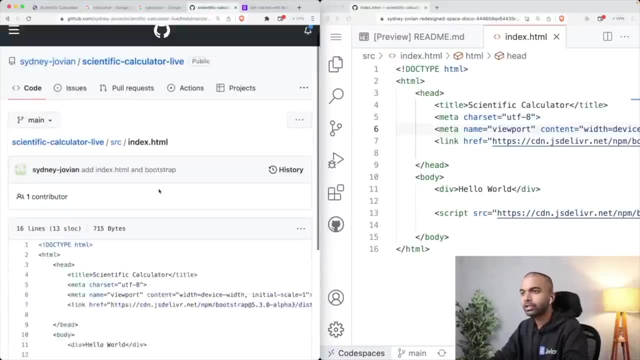 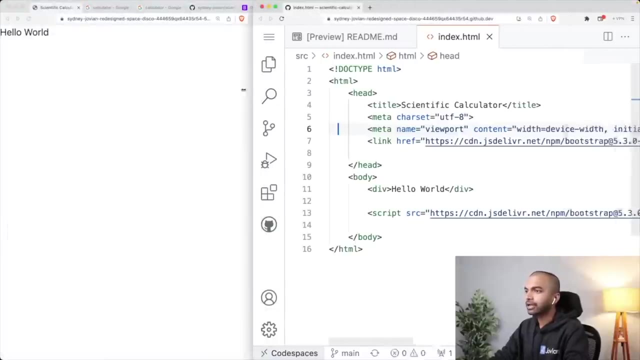 those changes back to GitHub. So GitHub makes this workflow very simple, And now you can see that in this index dot HTML file you actually have the scientific calculator basic code that we have put up so far. All right, so with that, let us actually start building the scientific 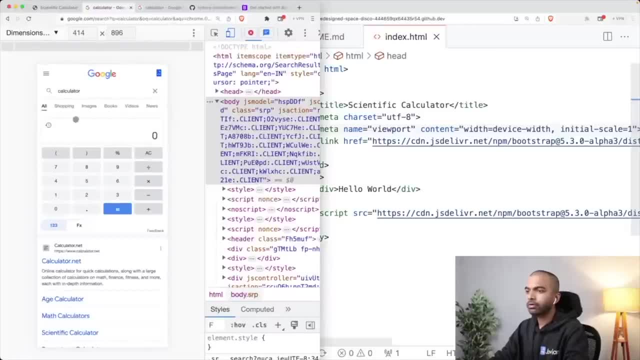 calculator. So I am just going to build piece out for now to begin with, And this looks like: okay, maybe I just want to put this in the center of the page somewhere, somewhere over here, And maybe I'll just put a title called: 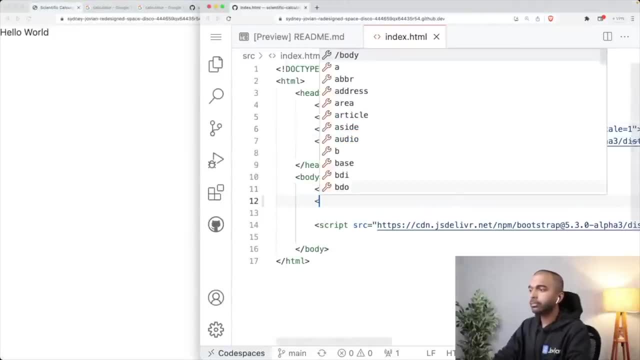 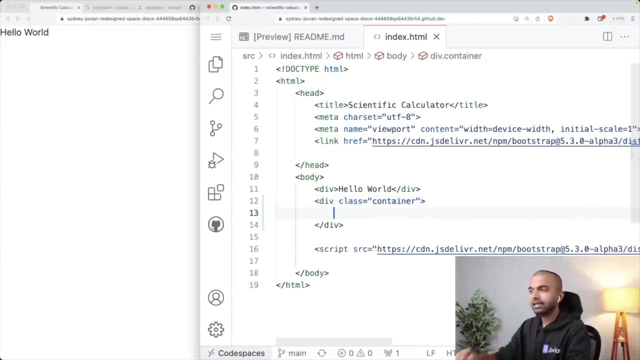 scientific calculator somewhere. So I'm going to start by creating a bootstrap container. So I'm going to create a div with the class container And what that does is that creates this nice div which is always going to remain horizontally centered within the page. And let us inside this: 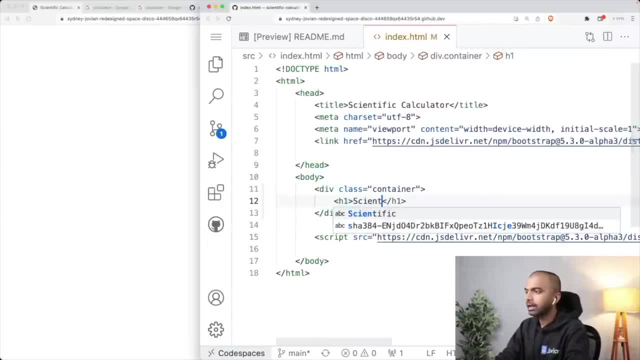 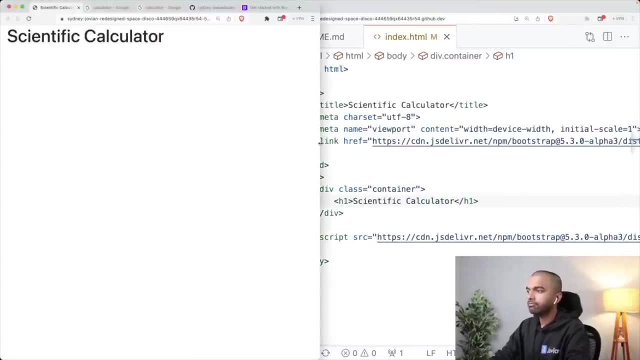 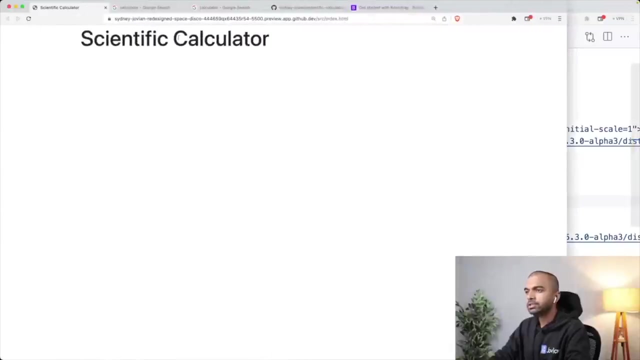 div, let us put in an h1 or a header tag And let's call it scientific calculator. Okay, perfect. So now we have this scientific calculator thing over here And this is looking fine. I and you can also see that the container is actually centered on the page. So that's why this is. 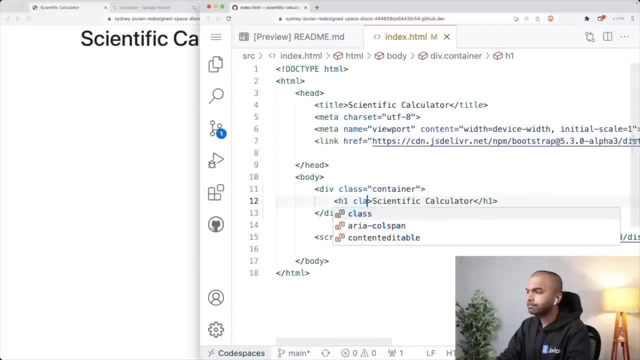 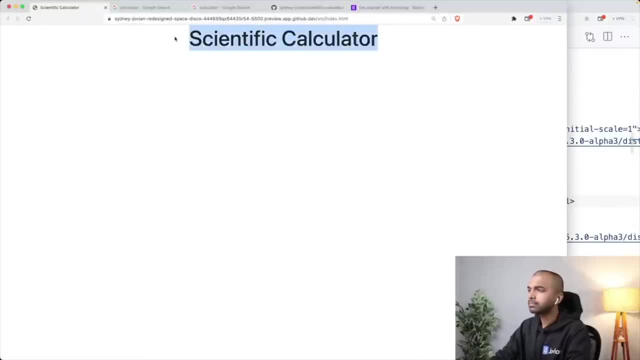 centered. But I could also just add text center- the class text text center- on the header itself, so that this header comes right in between. Okay, I could also control the font size if I wanted. maybe this is too big for me, maybe I don't want. 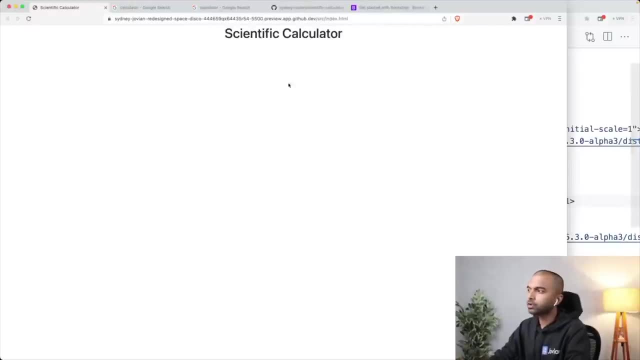 something so big. Well, actually I'm not. I'm a bit zoomed in And that's why maybe it appears a bit too big. I might want to add some space above, And that is where you would normally write some CSS. you would say margin top 32 pixels, or something like that, And again, bootstrap provides. 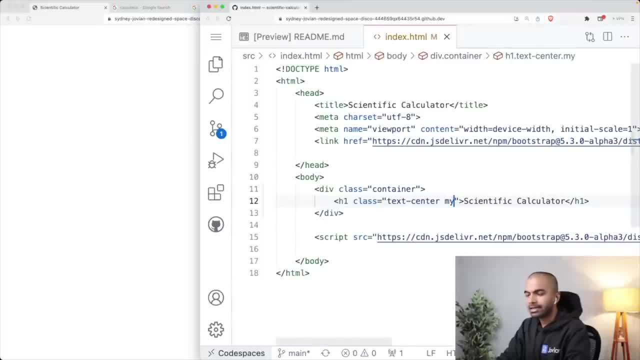 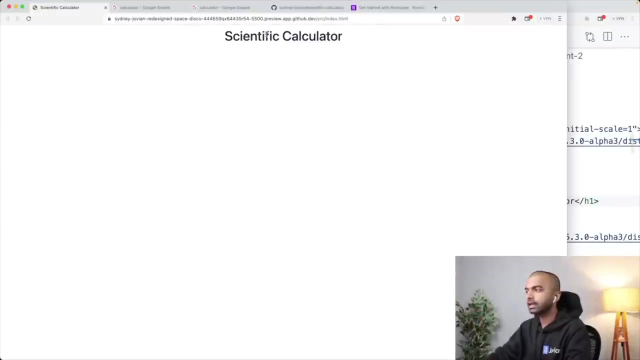 some simple, simple classes, utility classes, where you can say something along the lines of my or empty, which stands on margin top and you can say empty too, And it has like a pre configured sets of margins So you can say 123405.. And that is going to control the margins. Let me try empty. 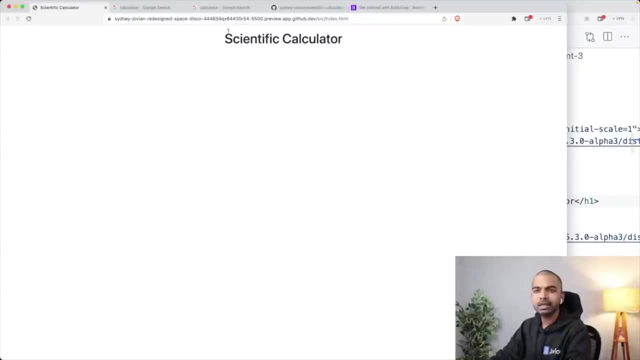 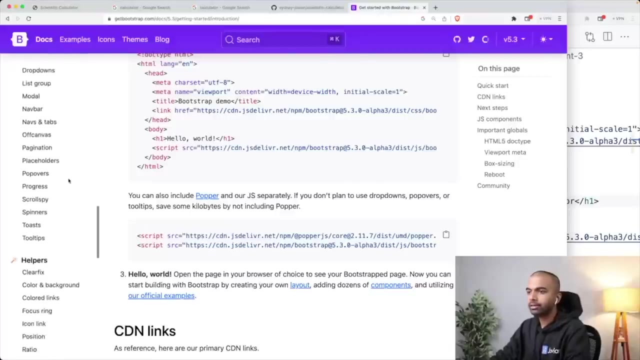 three, Yeah, so I think empty three, that is the amount of margin that got added here. That looks good, Okay, So that's the utility of bootstrap And you can check out all of these classes simply by looking up the documentation. So there are these utility classes for spacing And you can see a. 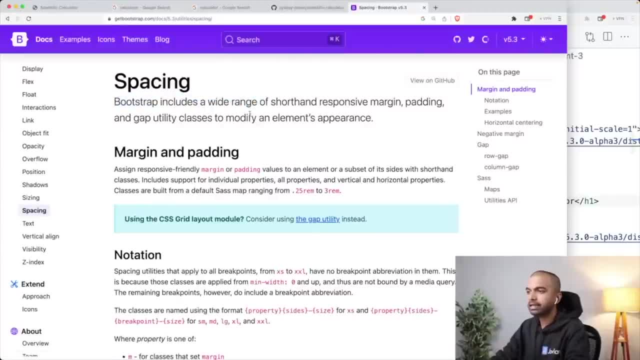 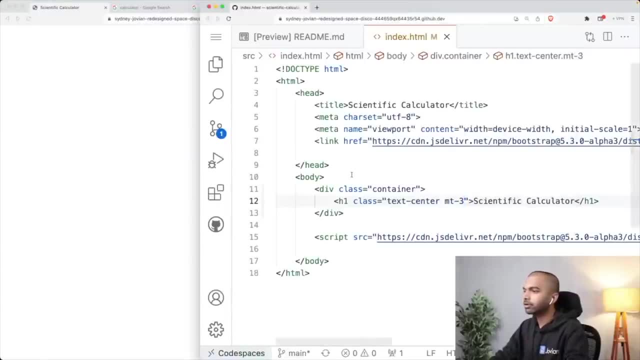 bootstrap includes a wide range of classes of shorthand, responsive margin, padding and gap utility classes, And you can do something like empty one, empty two, empty three, So I'll let you experiment with it. This is not a bootstrap tutorial, But the idea is we've just spaced things out a little bit. we've centered this on the page. 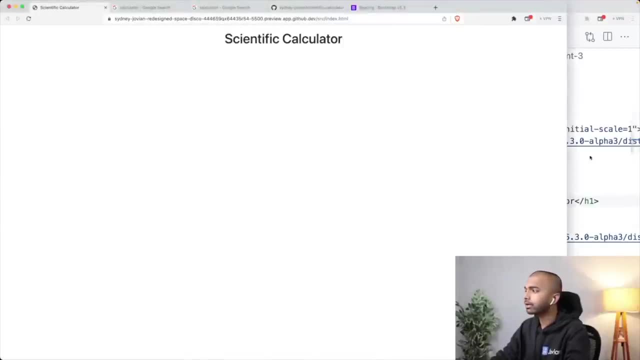 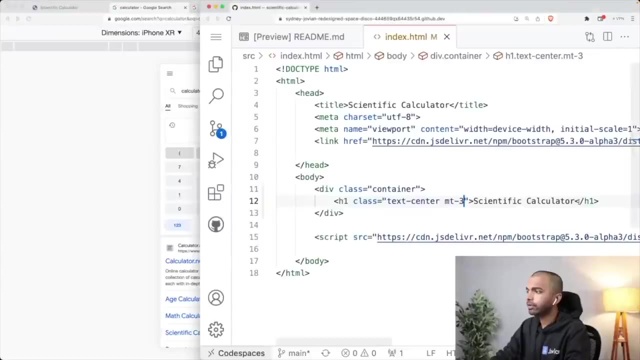 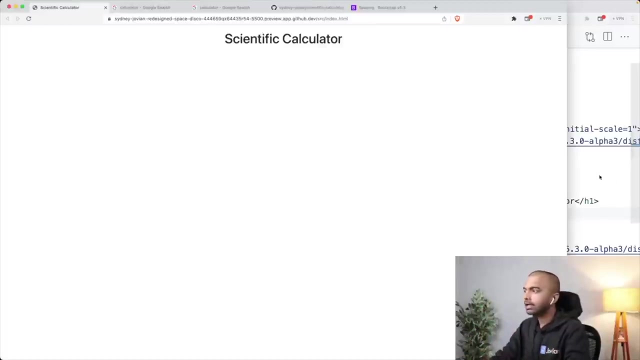 And we have now put some space above our title And let's start building this. Let's start building this actual calculator. So I'm going to put this calculator inside a card, a bootstrap card, because that would be a nice way to kind of contain the entire user interface of the calculator. because my page is 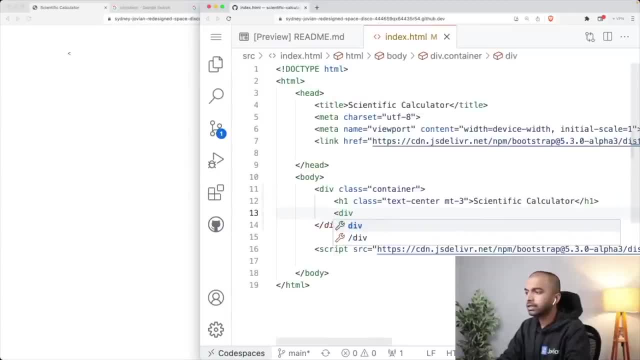 largely empty. And the way I'll do that is: first I will create a row. So in bootstrap, whenever you're creating a responsive layout, you start by creating a row, And in that row I am going to now create a column. Okay, and in this column, so maybe let's just look at the row And let's just add a. 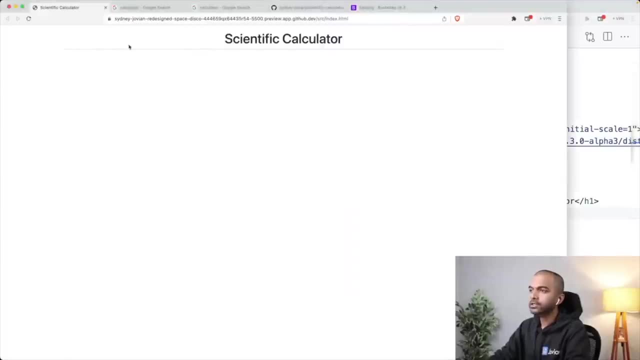 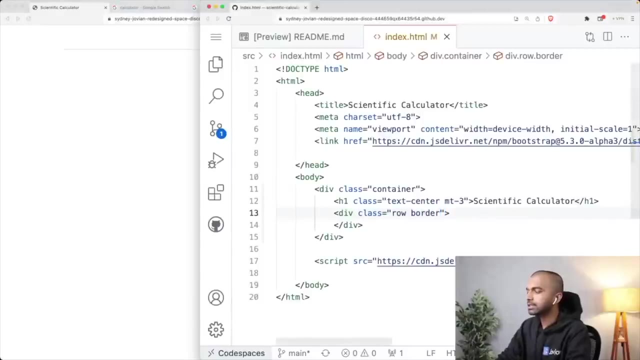 border to the room so that you can see what the row looks like. So right now we have this row, And this row takes up all the space from this end to this end. that's a lot of space. I probably don't need that much space, So I'll do. 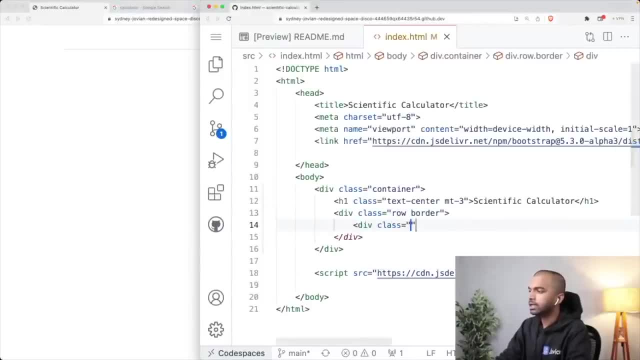 something about it, But let me now add a column to it. So let me add a column And let me make this maybe just six. let me make its width six columns long. So in bootstrap there is something called the grid system, So every row is split into 12 columns And you can create a div spanning six. 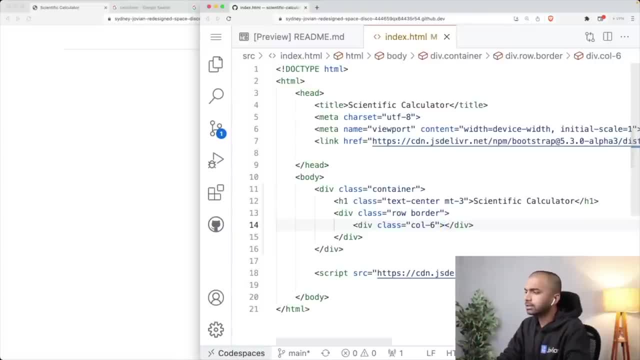 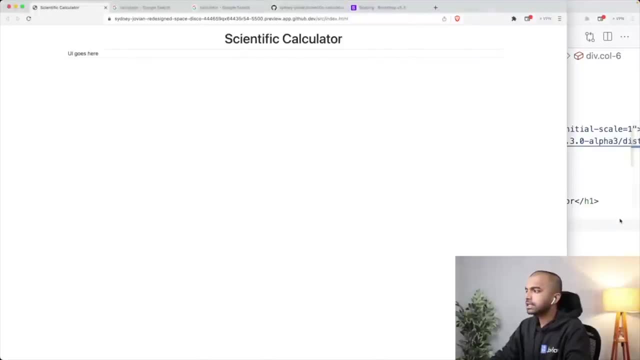 columns. So this is where my UI, My UI, is going to go. So I could say: UI goes here, All right. So now you can see if I add another border around this. you can see that now we have this row of content Once again. I'll zoom in for you. 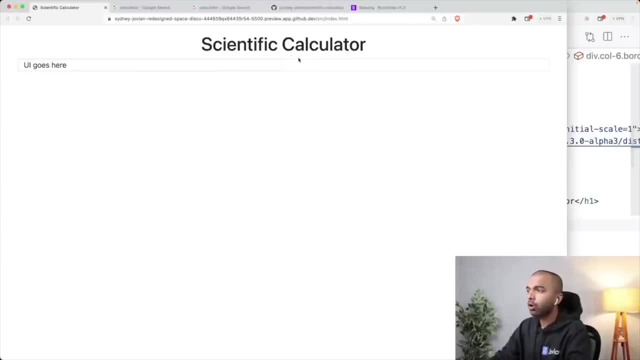 so that you can see clearly what's happening. But yeah, you can see that now we have this row of content And in that row of content we have this column, this one, this one div that covers six columns out of the 12.. I want to center this div. I don't want it to take up the entire width. 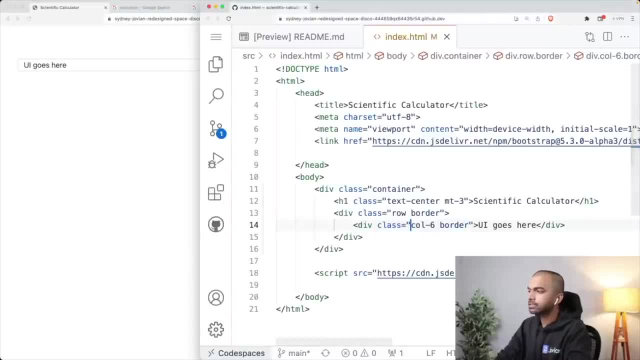 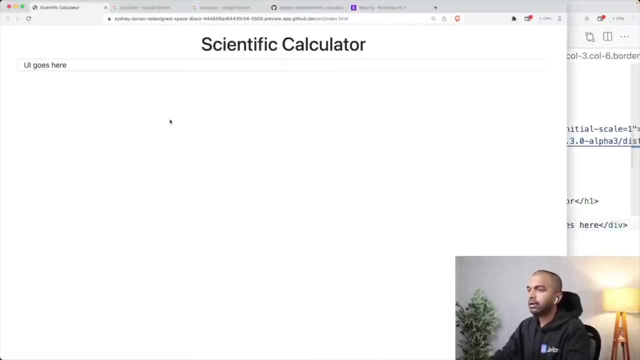 but I want it to center. So that's where I can say something along the lines of offset, call three. And okay, that doesn't. Yeah, I guess it's just offset three, Yeah. So now what we've done is we have said that we have a row, and the row spans the entire width of the container, And 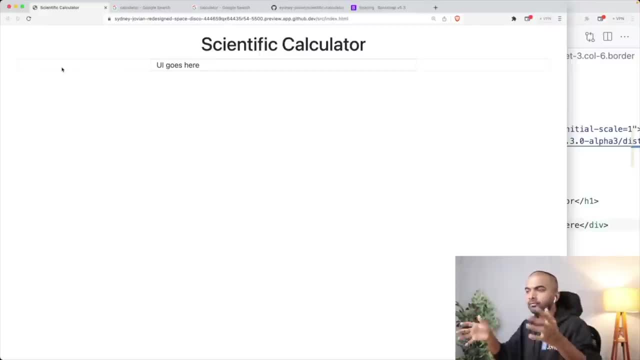 in that we are going to create a column as a div which spans six columns, But of course it's not going to be a div, it's going to be a column. So we're going to create a div which is going to leave three columns on the left, and then it's going to create a span six columns, And 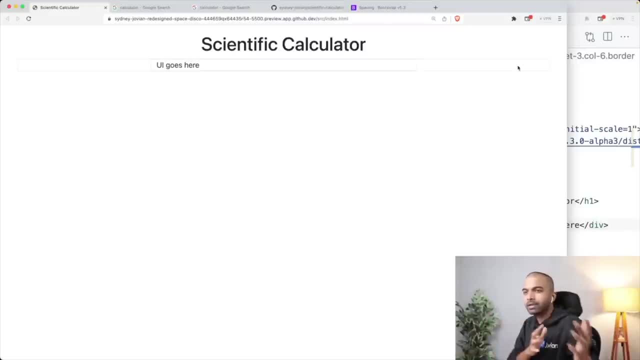 then, of course, three columns are going to be remaining on the right. Okay, so we've left an offset of three columns, we are taking up six columns, and then we have three more columns on the right that we, that is, that we've centered this user interface on the page, Alright, so 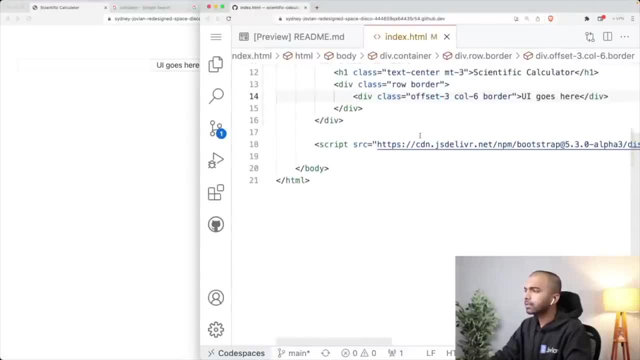 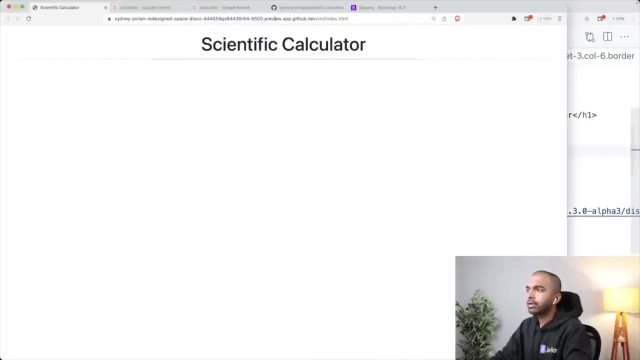 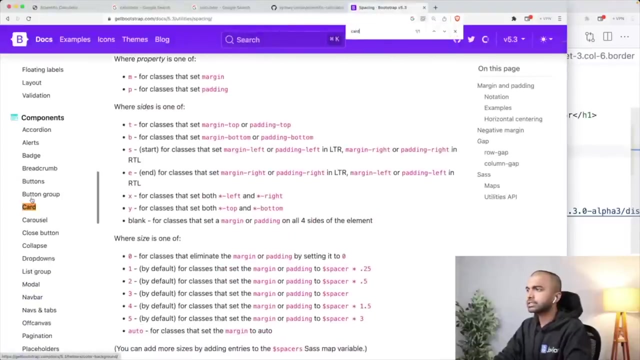 so far, so good. This is looking fine to me. Now let us start adding some of the user interface for our calculator. Now I'm going to use a card to create the calculator, just to have a nice. Let's see. let's just search for card. 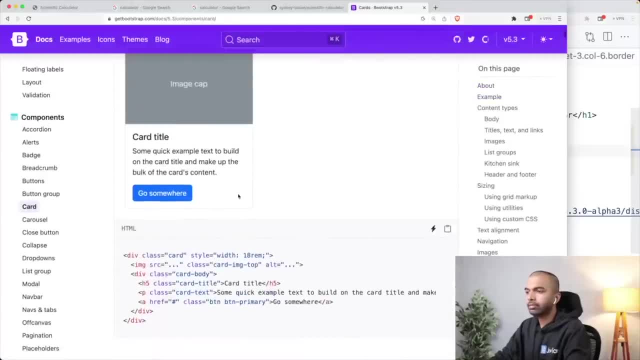 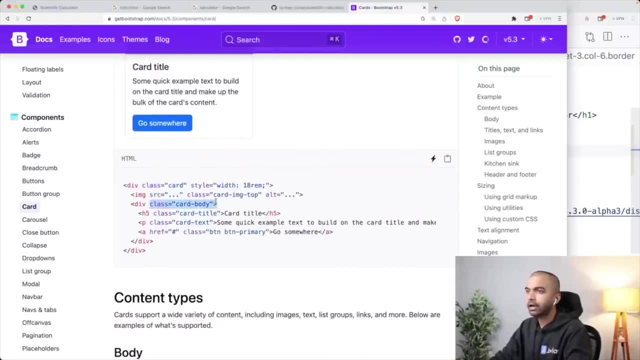 So just to have a nice border around my calculator, around my calculator, I'm going to use a card. So here's what we can do: we can create a div with a class card and then we can create a div with a class card body. So let me just quickly do that, Let me get rid of these borders. 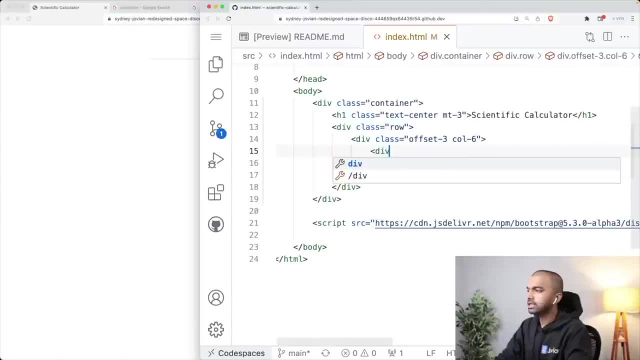 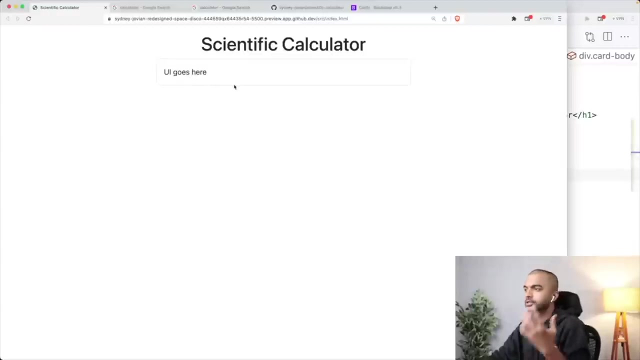 And let me get rid of these borders, And I'm just going to say div class equals card, And I'm going to say div class equals card body And my UI goes here. Okay, so we're getting close. So you can see that by using the card component. 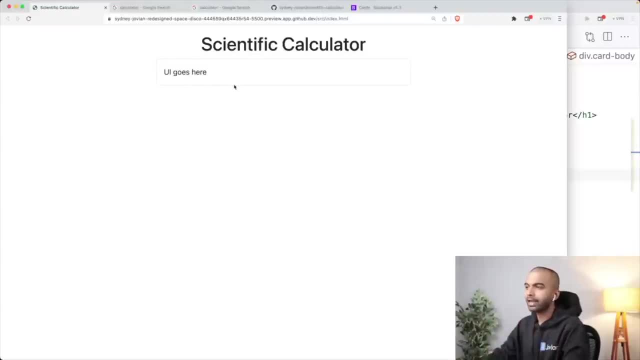 from bootstrap again. just look it up, just look at an example, you'll get it. Now we've created this nice card And inside this card we have this nice user interface that we can now start building. Okay, And now let's start by creating. So what's the first thing here? the first thing is: 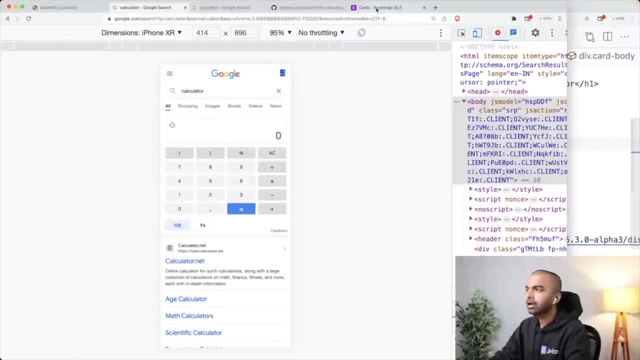 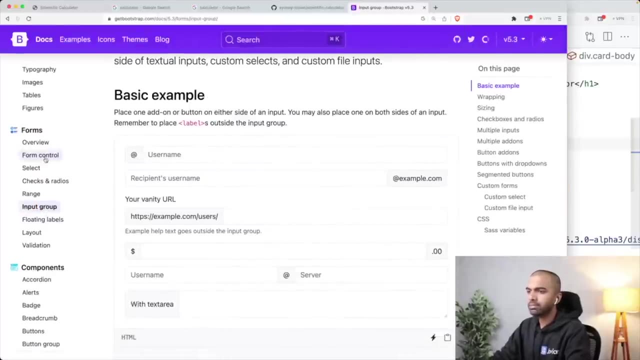 input box right over here. So let's start by creating this input box. How do we create an input box? Let's search for input. Okay, looks like there's something called an input group which we can use, or maybe even like form control. I think we need something like this. we probably 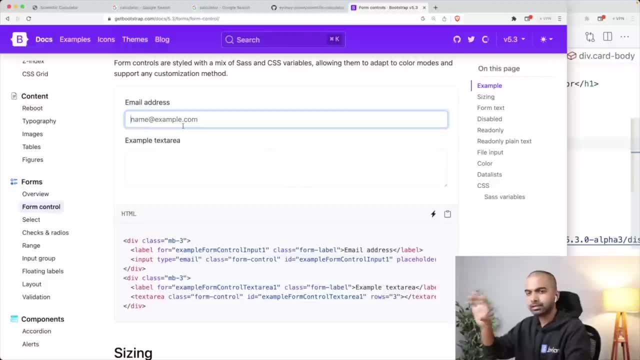 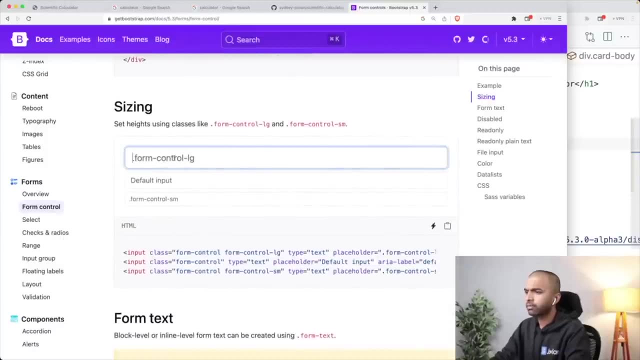 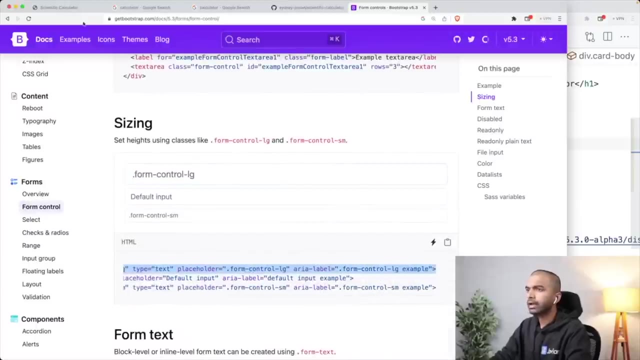 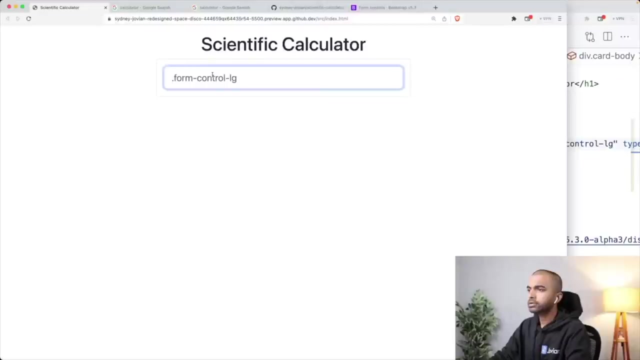 want to just show the output of the button clicks the current expression in an input box like this. So I am going to use- I think this looks good- form control LG. So maybe I can just use this. So let me just copy this form control LG and come back here and paste that in here And, yeah, that looks good to me. 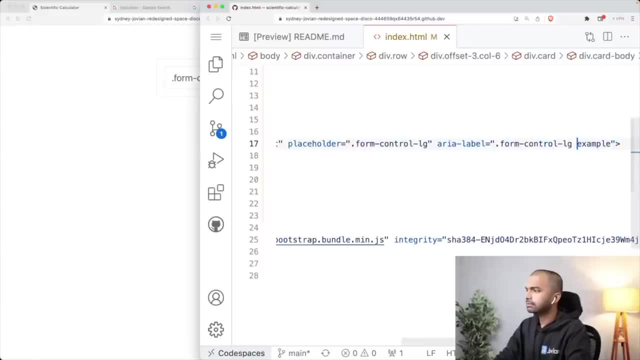 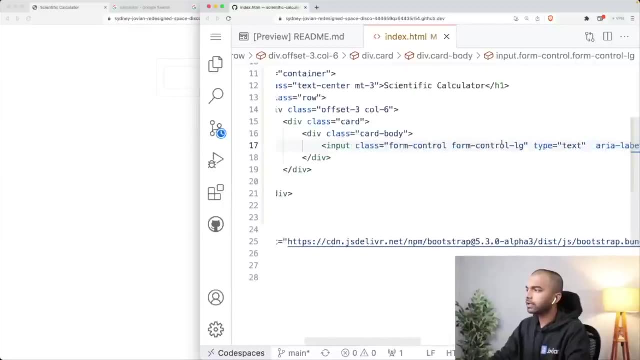 Of course I probably don't need. I probably don't need this placeholder over here, So let me get rid of placeholder. So you can see we have an input of the type text and it has the class form control and form control. LG to LG simply means large, So to make it a little bigger, 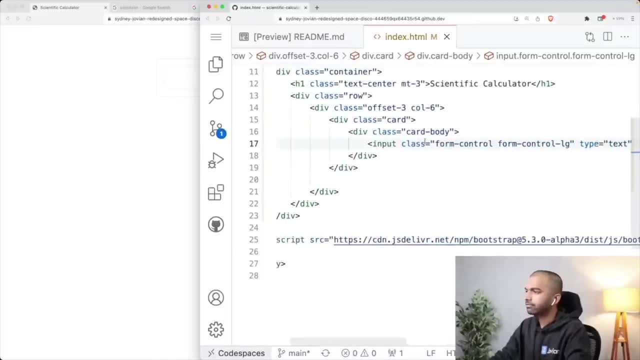 finally, we have a bunch of other labels that we might find useful. Okay, so now we have form control LG. I'm also going to make this read only because we don't want to be able to edit this directly, So I'm just going to make it read only like that, And we only want to edit it based on. 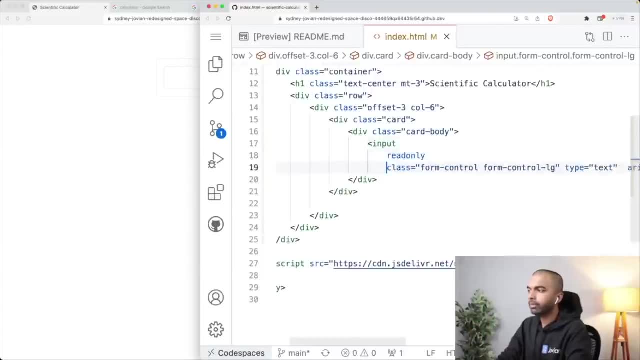 the content that we put from the buttons that we click. okay, and that's going to come up soon. All right, the last thing I'm going to add here is maybe an item, Because so I'm just going to give it an ID calc display, And because this 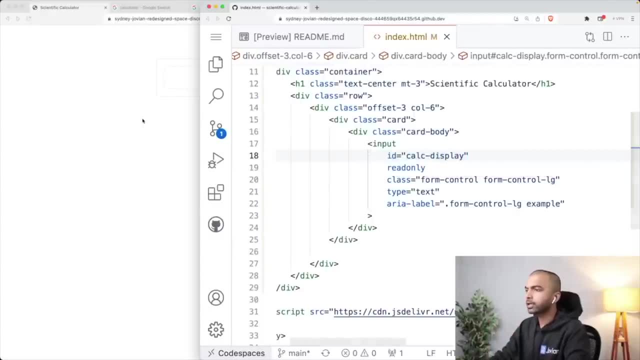 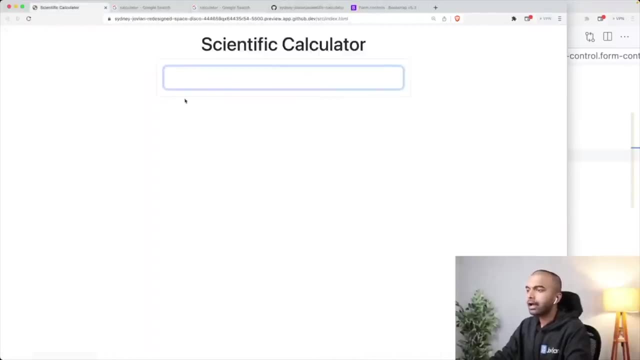 ID is going to be used to actually set the value of this particular field over here. Okay, so now we have this field, something like this, not exactly this, but close enough. Now we need to start adding some buttons. So we have all these buttons, okay. brackets percentage. 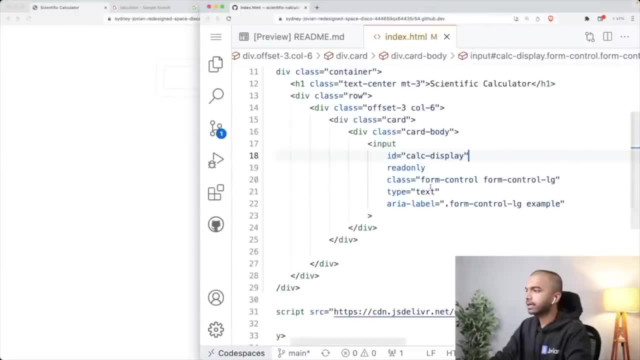 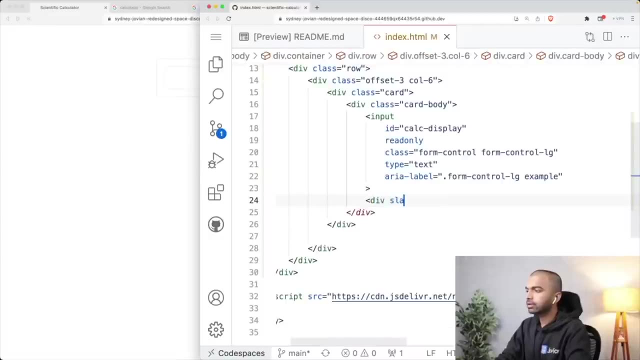 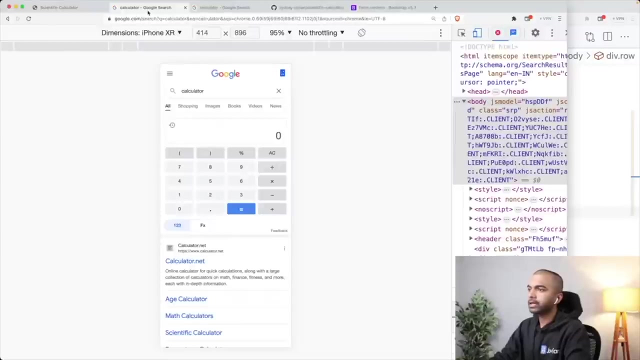 AC, 789, etc. So let's start adding these buttons. So, to add these buttons, I am once again going to create another row. So I'm going to say div class equals row. Okay, and let's add the first row of buttons. 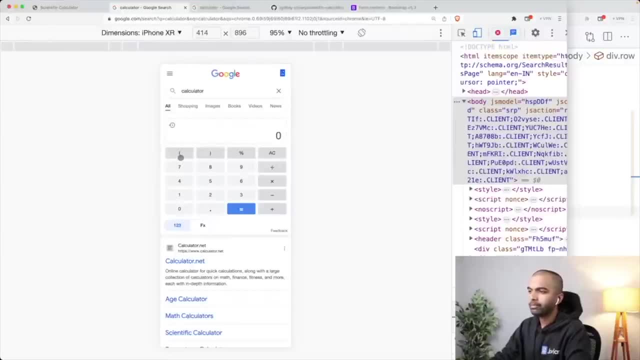 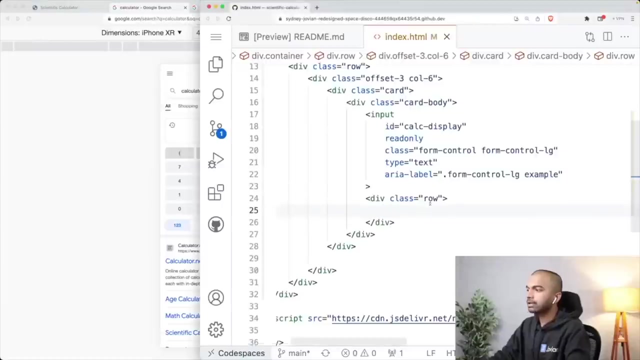 here. So the first row of buttons is: I'm going to use the BTN or button tag, And each of the buttons is taking up one fourth of the space. So remember that every row has 12 columns inside it. So that means each button is going to take up three columns. So maybe first let me create a div. 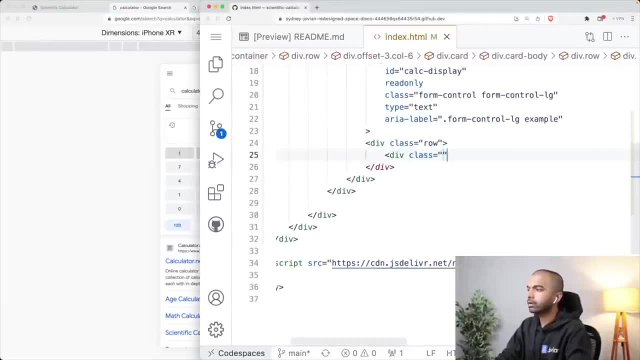 with three columns. So div class equals row And that's going to take up three columns. And inside this let me put in a button. Now, again, there's a way to put in buttons in bootstrap There's. there are some helper classes, So I'm 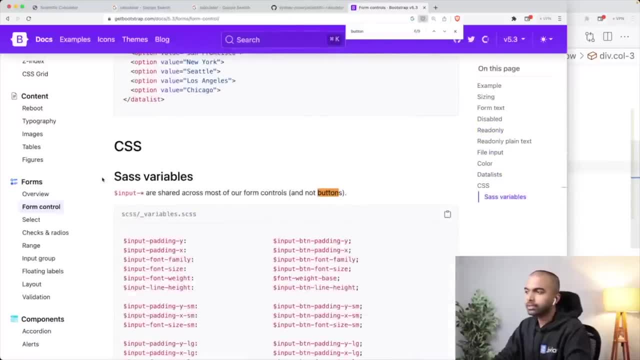 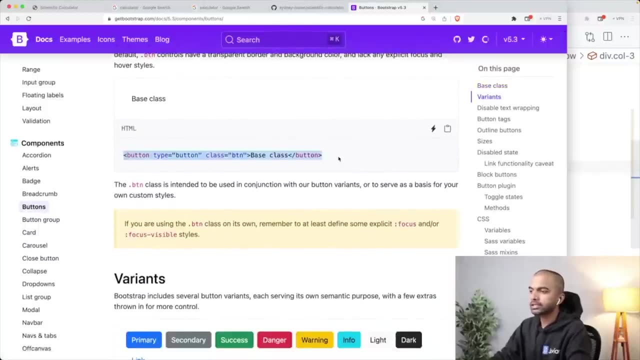 just going to search for button right over here. And again, we're going quickly because this is not exactly a bootstrap tutorial. But you can go to the documentation. you can see what buttons look like. This is what buttons look like. I don't want a base button maybe. I want a button like this. 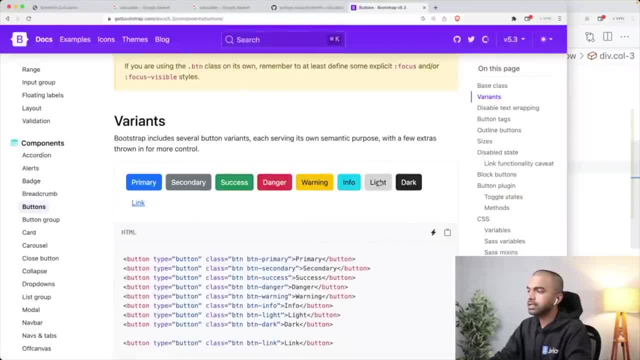 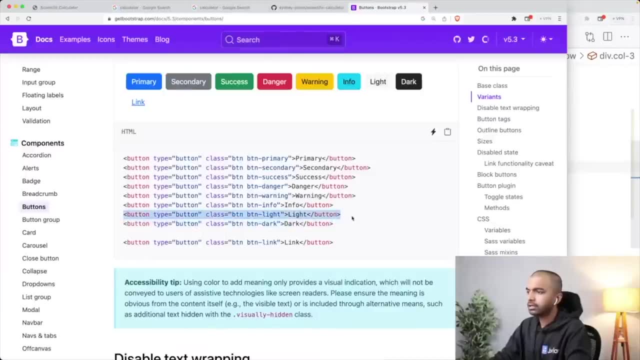 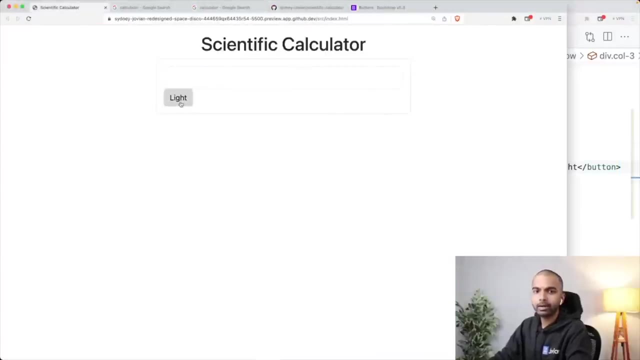 because that seems to be the color that is used in most of these buttons. So I'm just- I'm just going to use BTN light or button light. Let's grab that- Okay, button type equals button BTN light- And let's just paste that in here. And, yeah, looks like we now have this light button, So that's. 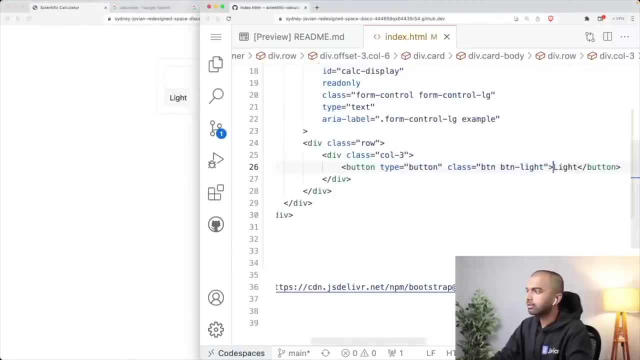 good. Of course we need some spacing around it. we maybe need to add a border around it, So let's fix that in a second. But at this point let me add one button here, So the button here. is that okay? so my buttons looking fine, And let's add maybe a couple more buttons And then we'll fix. 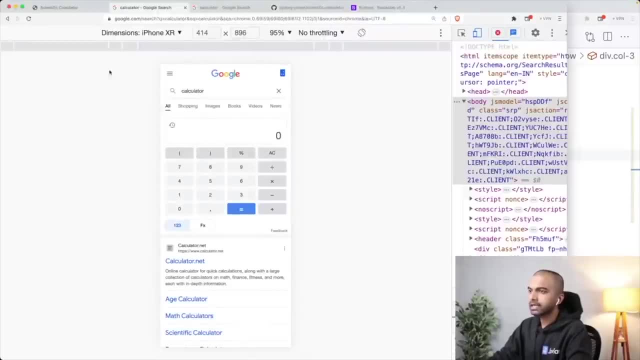 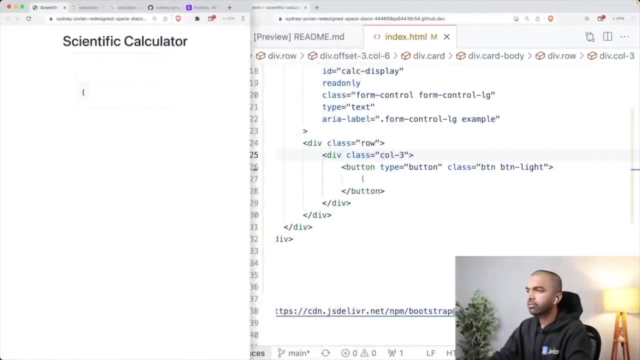 this spacing, etc. So we have another closing bracket, percentage and AC. So let's come in and fix those buttons. Okay, this is interesting Now, when we make, when we reduce the size of our scientific calculator, of our browser, that is going to squish the calculator a little bit. 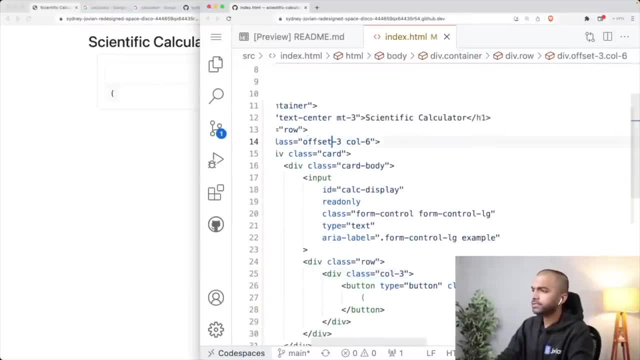 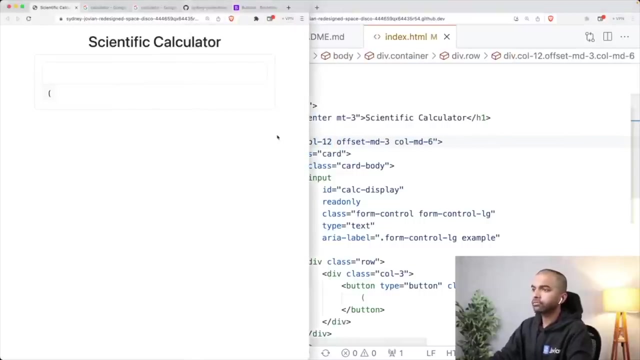 So maybe we can do this. we can say offset md3. And call md6. And for small screens we can just take: let it take up the entire space called 12.. Okay, so for small screens it takes up the entire width of the container, the. this is the. 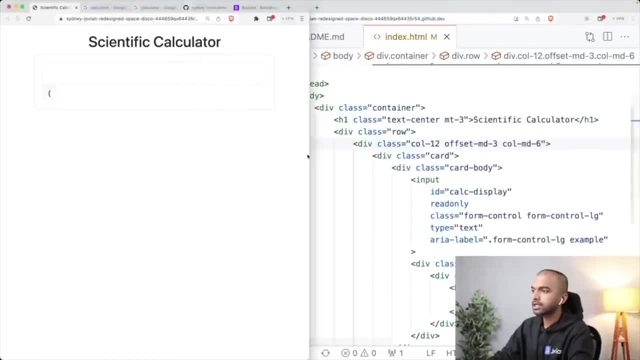 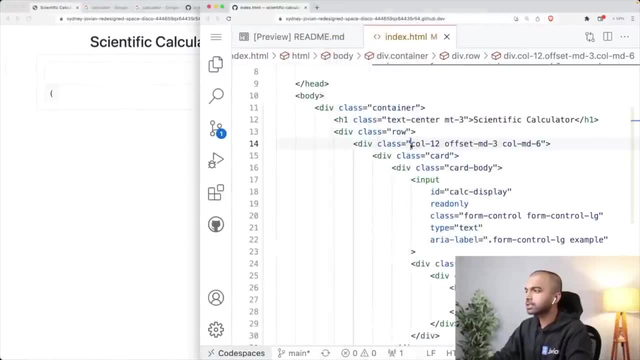 the div wrapping or the column wrapping the card. So for small screens it takes up the entire width and then it shifts into a smaller width later. for empty screens, Okay, and we can adjust this further towards the end, But for now this is fine. 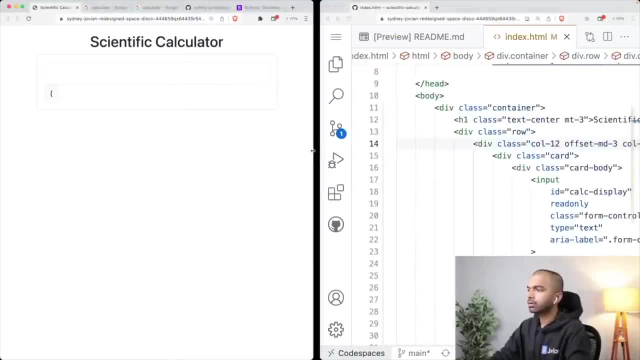 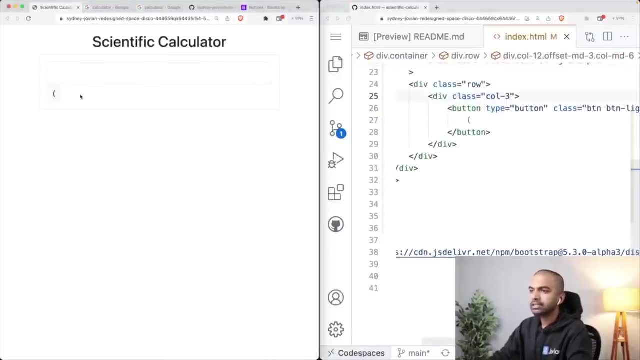 Alright, coming right back, we need to add a few more buttons, But let me just improve this button slightly a bit. The first thing I want to do here is: let's put one more button and then we'll see what we can do about it. So the first issue that I'm running into, that this button is not really 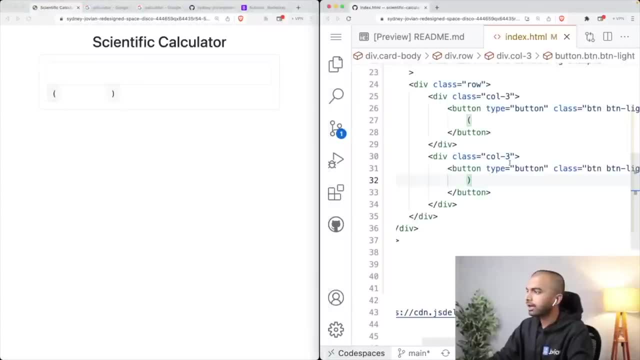 taking up the entire width of the column. maybe it should, So I could just come in into the button. And let me just go into the button and say w 100.. And w 100 is a helper class within bootstrap that makes the button take up the 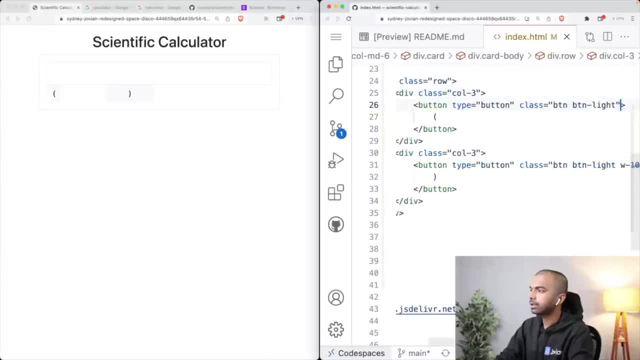 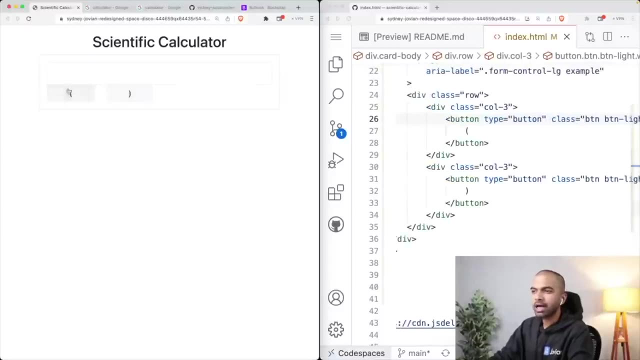 entire width of the column. Okay, let me add that here, the w 100.. Let me add that in here as well. So both my buttons have width of 100.. So that's good. I think buttons can also have a margin top. 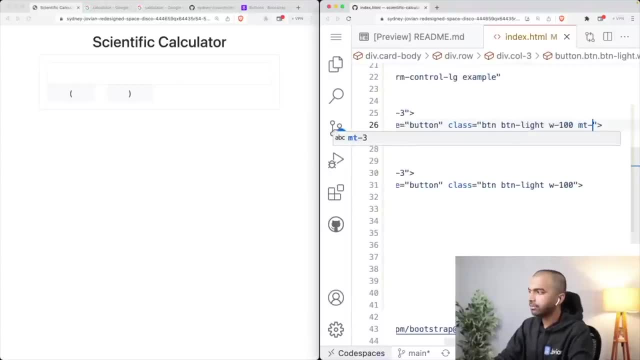 probably. So let me add a margin top here. So let me say empty one or empty two. Okay, empty two looks good. So now there is some top margin that we have added. Let me maybe also add a border to these buttons because it'll be nice. So let me add a border to these buttons because it'll be nice. 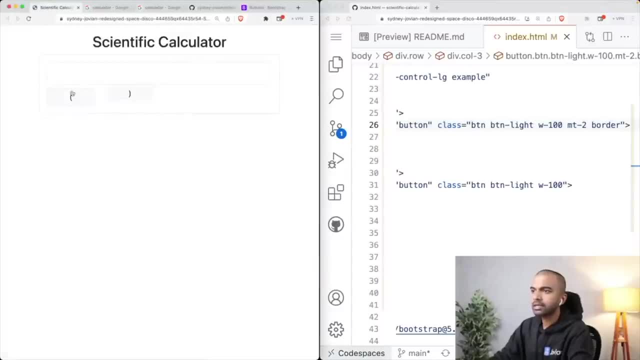 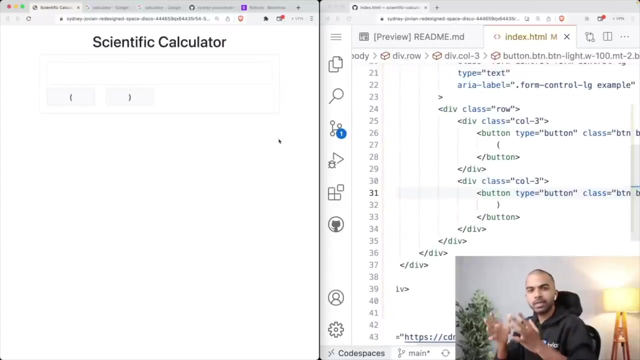 These buttons seem to have a border around them, maybe, So let me add a border to this as well. So let me add empty to border. Okay, the button is looking good. I think the space between these buttons is too high. Maybe I can reduce the space- And this is a default space- between the columns. 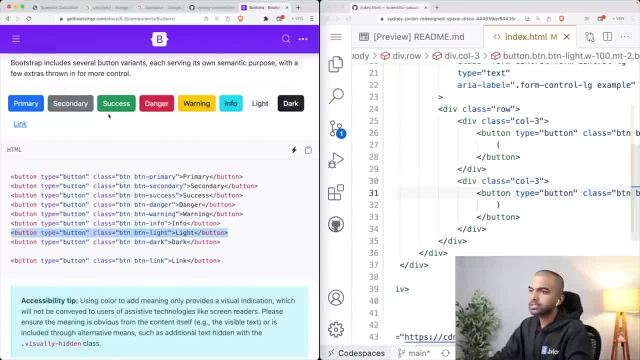 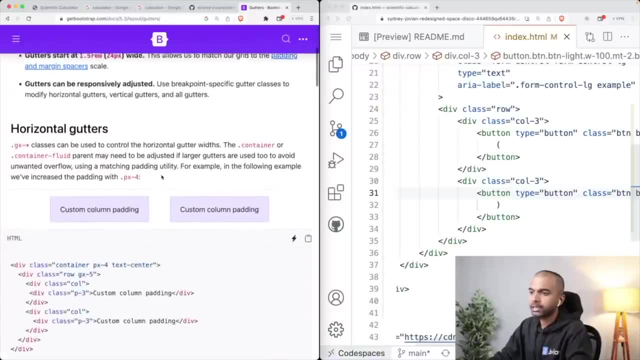 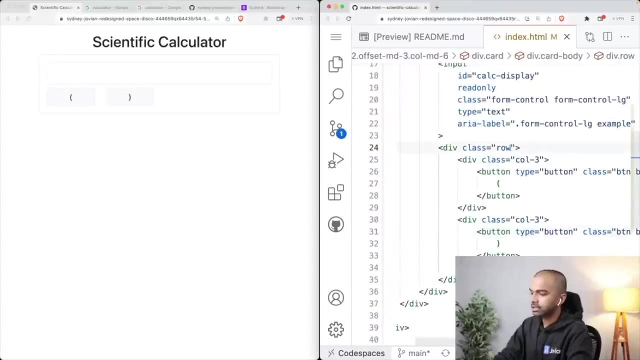 within a row And you can control the space between columns using something called gutters in bootstrap. Again, that is done. I'll let you explore this. But the basic idea here is you can use these GX and GY classes to control the amount of space between columns. So I'm just going to come. 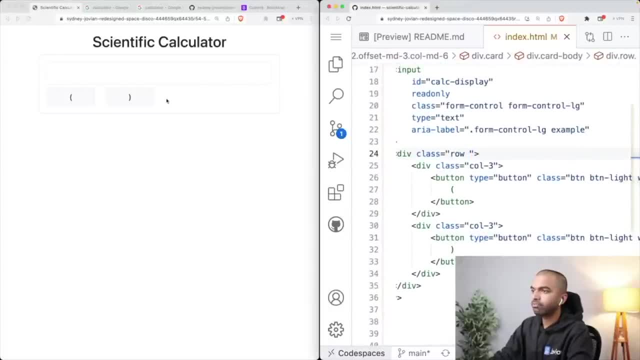 into them. come into my row here, which can, which is the row of buttons that I've created, And I'm going to say GX one, And you can see just as, as soon as I say GX one, the buttons become a little wider and the space between them reduces. Okay, so yeah, I've just added a bunch of classes here. 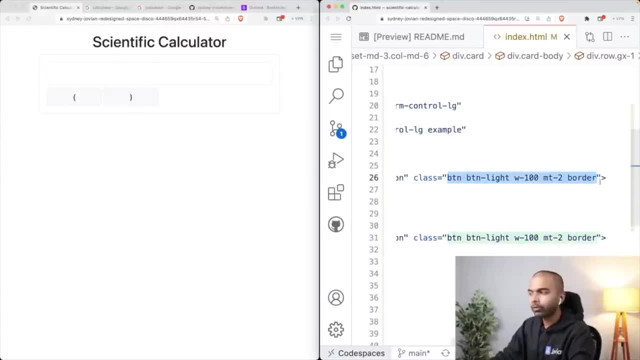 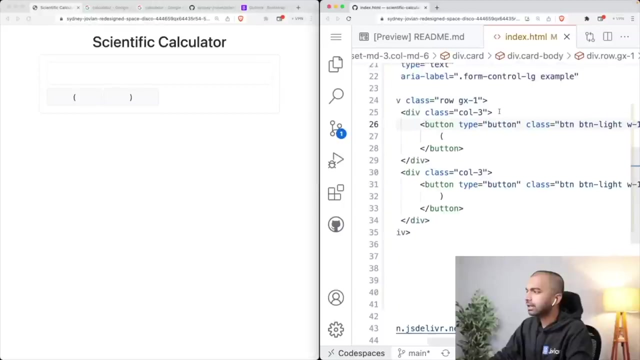 And you can always look up what these classes do. So I encourage you to do that, And I encourage you. what, exactly? what are the CSS properties that get applied here? Okay, All right, So now we have the button and we have another button. Let's take, and let's take these two buttons and add a couple more. 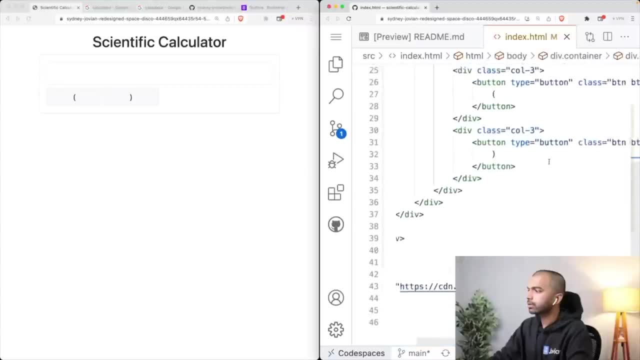 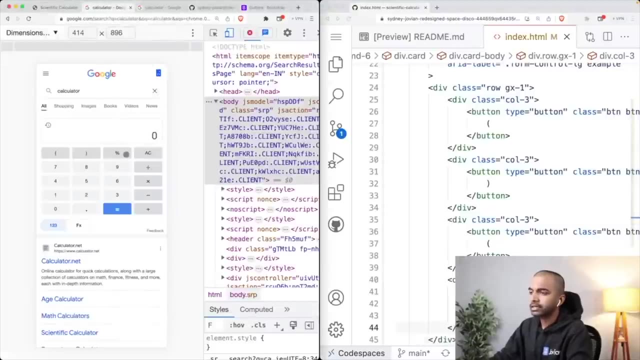 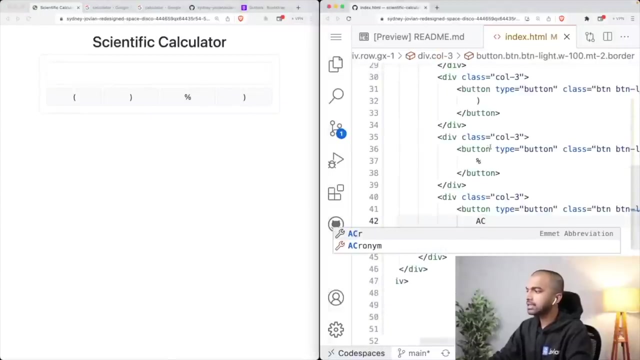 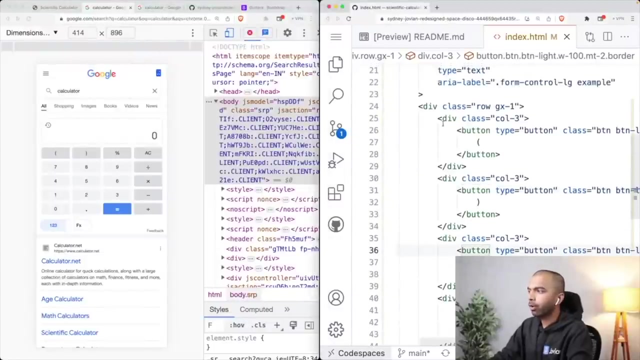 buttons. Oops, Okay, let's add. let's see what these buttons are. So percentage and AC are the buttons that we are adding here. So let's add the percentage symbol. Let's add AC. Okay, that's good. Now we want more buttons here, So one thing we could do is maybe create more. 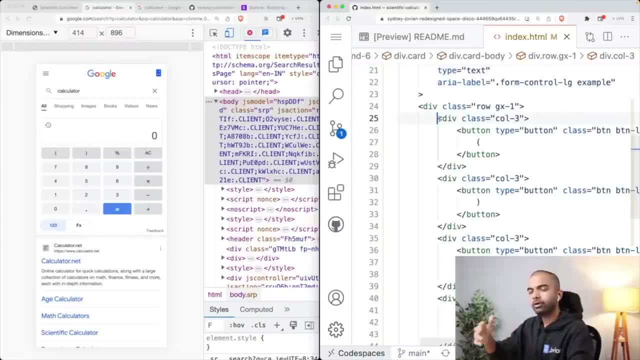 rows. we could actually create another row and then in that row add multiple columns. But remember that bootstrap has 12 columns within a row And if you try to create a div that does not fit within those 12 columns, it will automatically go to the next line or the next row. essentially it's going. 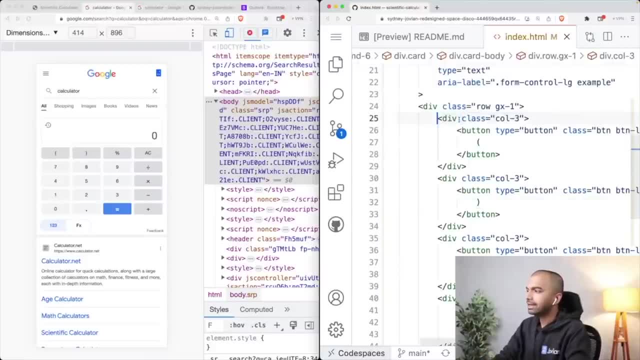 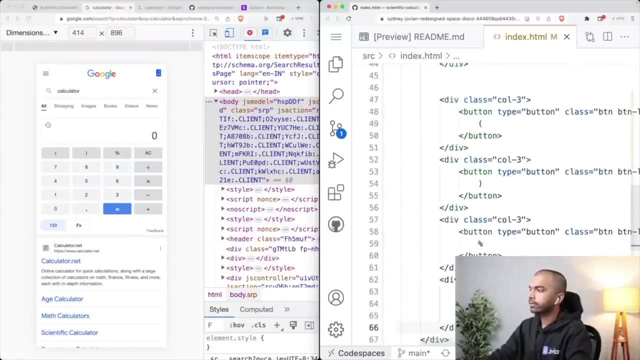 to wrap onto the next line, So I can. I don't actually have to create a new row. I can simply copy these columns And just create another set of columns right below it, And what that will allow me to do is I can then make it a little more flexible, maybe in my layout, But you don't have to do it this way, It's. 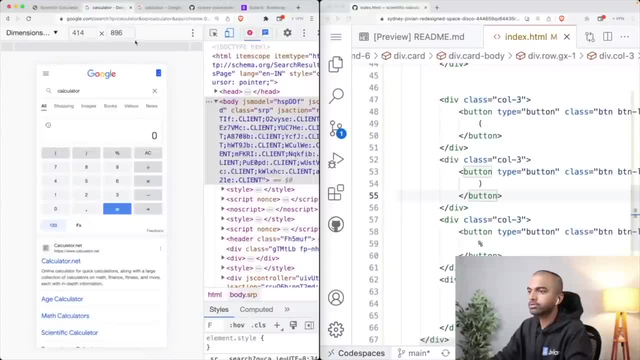 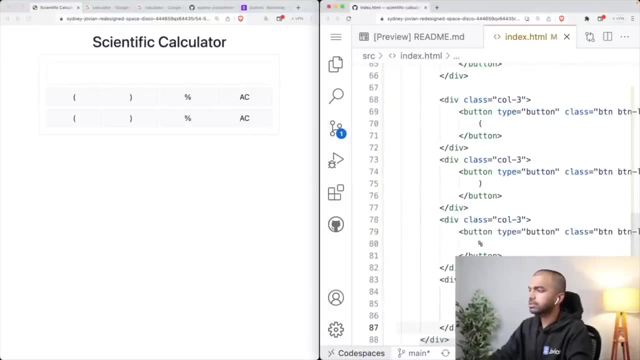 just an easy way to do it. Okay, so here's my second row of buttons. How many rows do we have? So we have 12345 rows, So let's add those five rows here. So I'm just copy pasting, I'm just 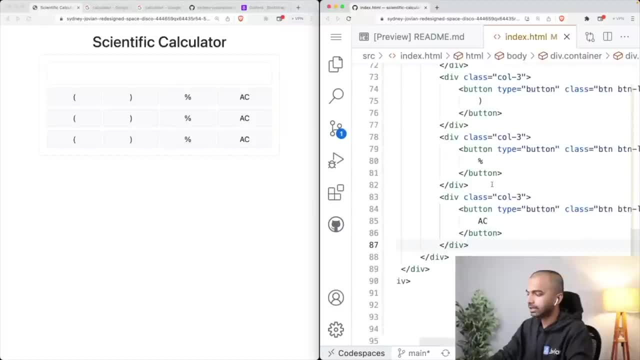 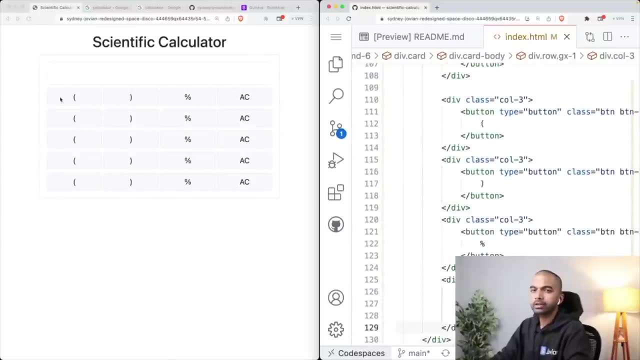 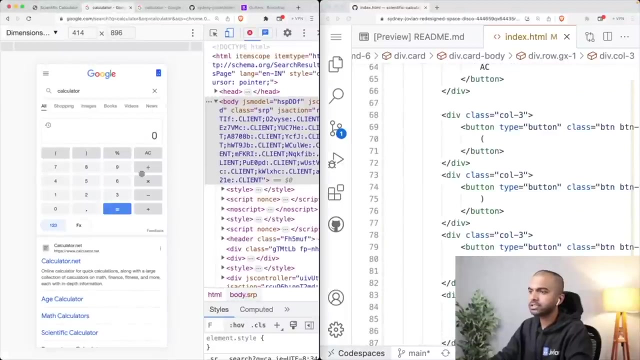 copy, pasting these four columns. are these four column buttons again and again: One, two, three, four And let's add one more set of buttons. Perfect, Alright. so now we've added a bunch of these buttons And let's maybe actually put in the value. So we have 789 and the division symbol. 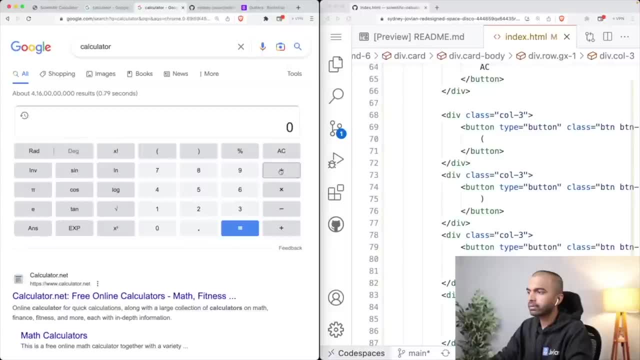 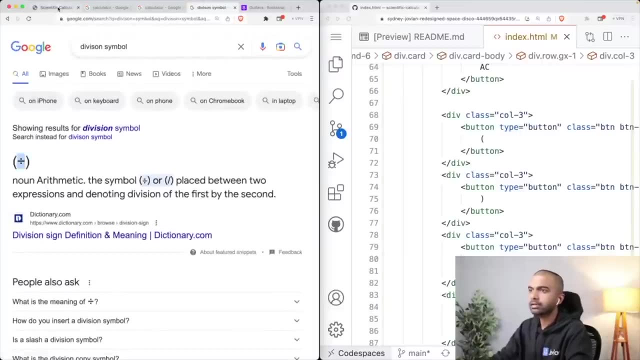 we should find a way to actually copy that division symbol. Let's find it. So if you just search Division symbol, you can actually find the symbol online. But anyway, let's first put it in. So this is the first row of data. So this is fine. Then this is the second. row of data or second row of buttons, And then let's add this new row. Now I don't want to do an additional set of buttons for this, But I want to start by doing this. So, first row of buttons, this is: 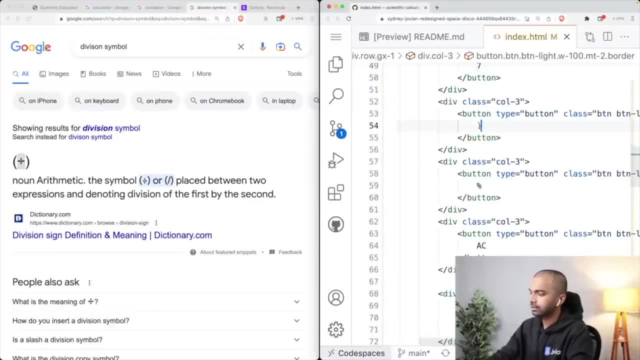 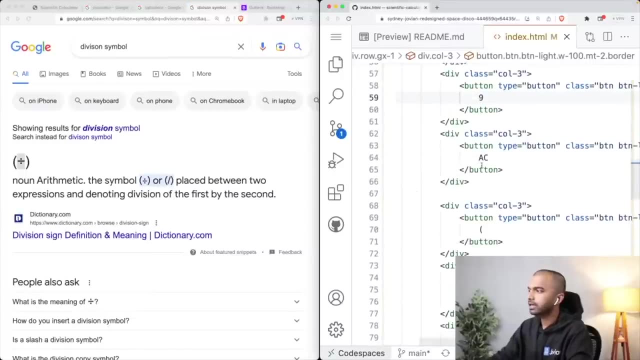 the first row of data, So I'm going to add this first row of data. So this is the first row of data. So I'm row buttons- let me make them 789- and the division symbol. So let's copy that division symbol and put. 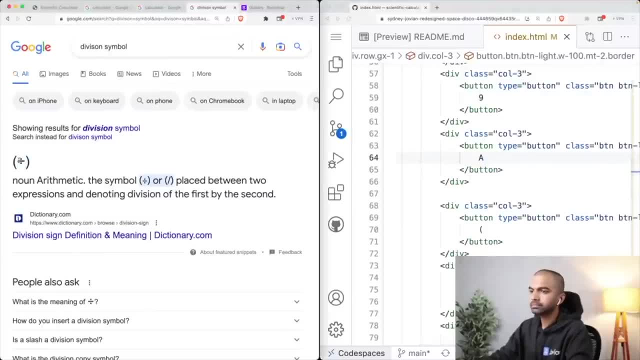 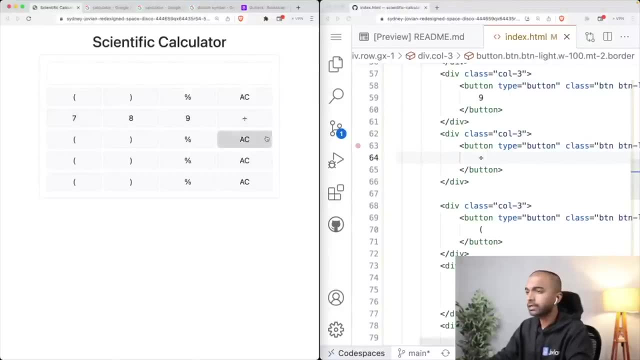 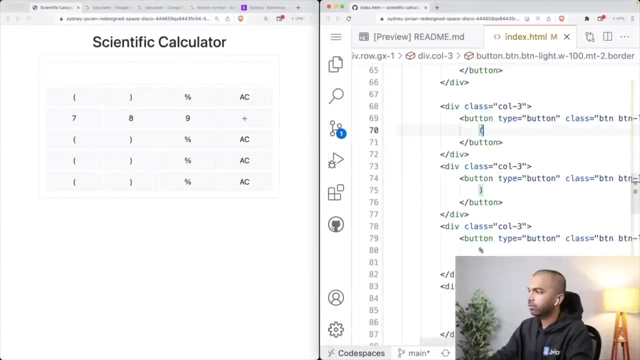 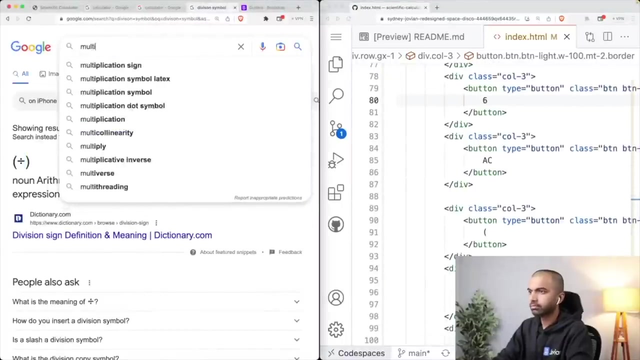 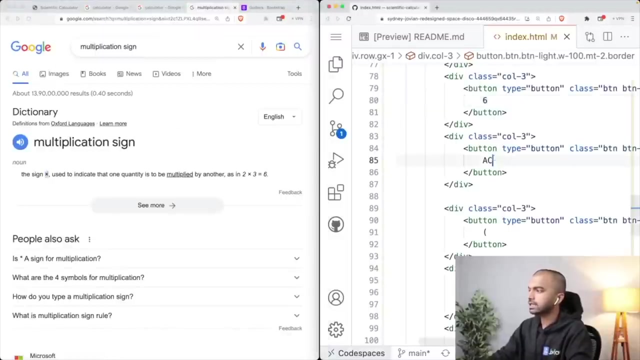 that in here. Okay, so now you have 789, division, Perfect. Then let us get that next row, that is 456 and the multiplication symbol. So let's get that in: 456 and multiplication symbol. Yeah, this is the multiplication symbol. So 456 and the multiplication symbol- Perfect, It's. 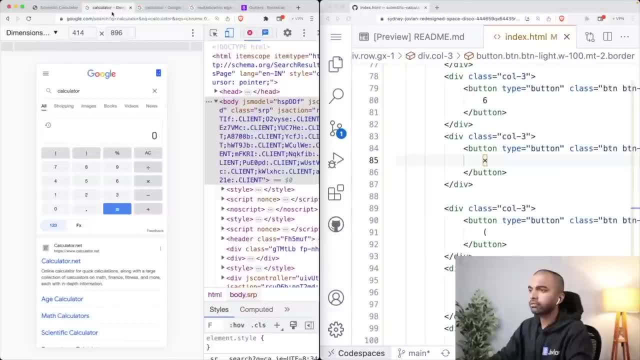 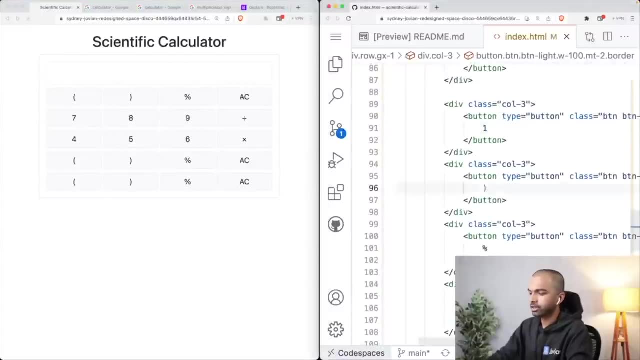 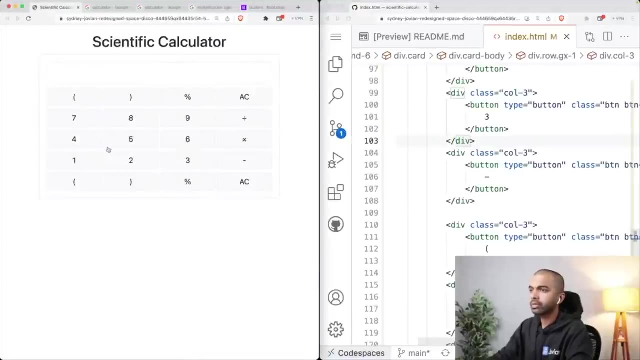 looking good. Let's get the next set of rows here. So 123 and the minus symbol. So let's get. the minus symbol is already present on the keyboard, So we don't need to change a lot here. 123 and the minus symbol. Okay, we've added the next set as well. Finally, we have zero dot equal. 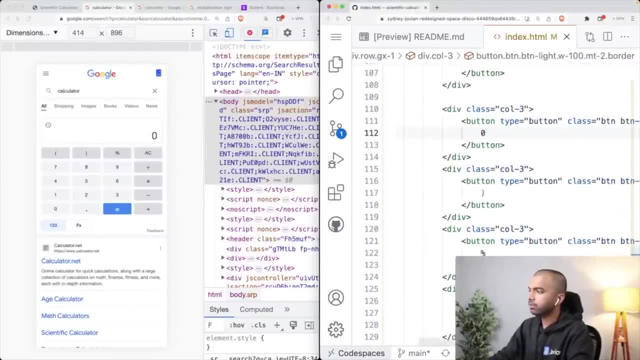 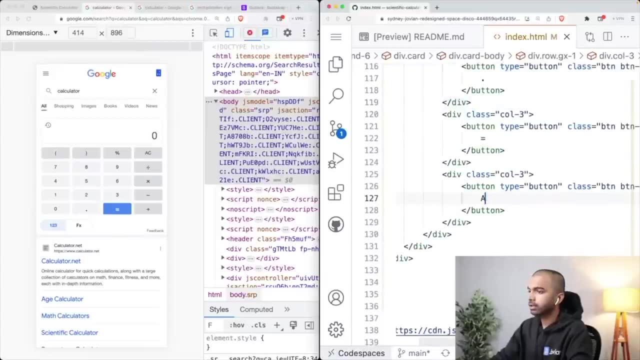 to and the plus symbol. So now we have zero, we have dot or point or percentage or decimal point equal to and the plus symbol. Okay, perfect, It's looking good. I think the equal to symbol can be made blue, And again, this we can do simply by changing the class here instead of button light. 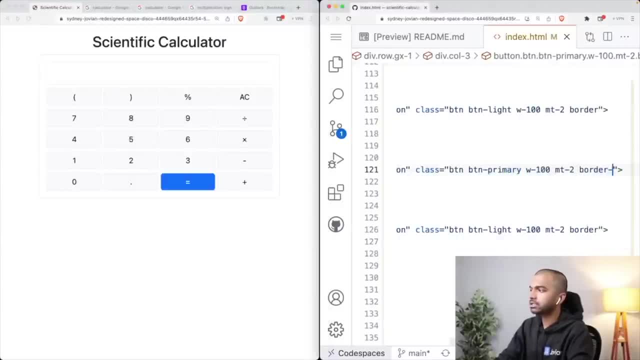 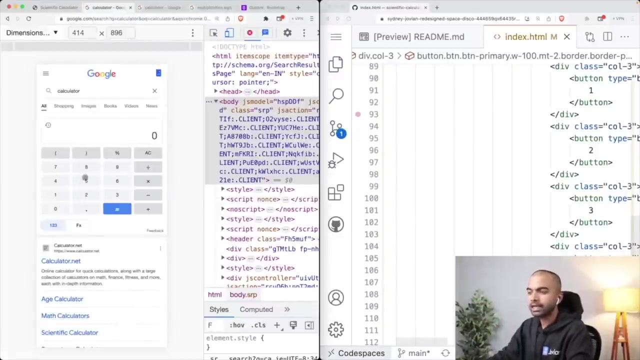 I could say button primary and instead of border I could say border primary, or maybe like border and then border primary, And that's going to give it the blue color. Okay, with that, we have implemented the basic user interface of the scientific calculator, right. 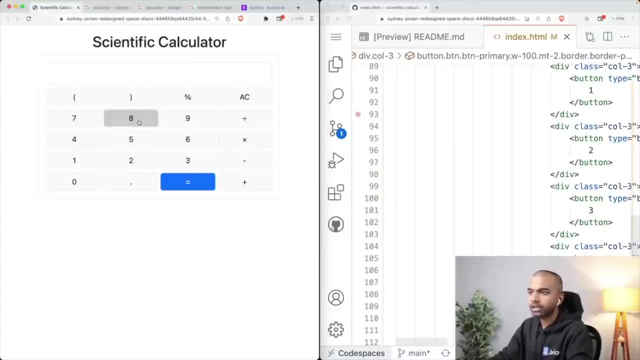 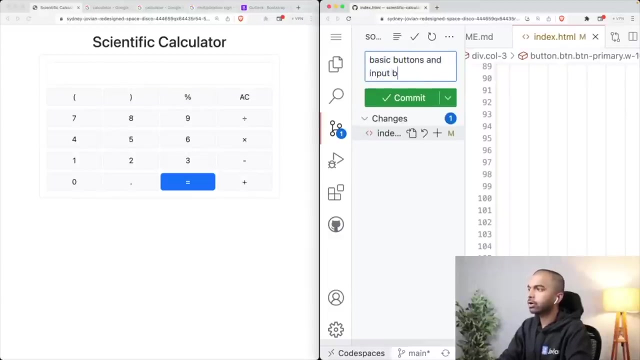 over here And we have. of course it's not working. yet none of the buttons actually do anything But a for 1520 minutes of work. this is not looking too bad, Okay, so let's go ahead and commit that. So, basic buttons and input box: Let's commit it And let us just sync it. 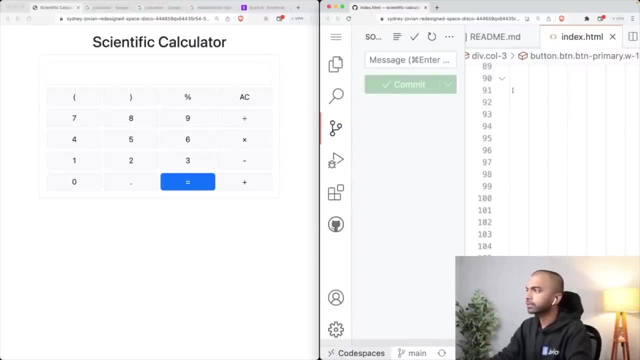 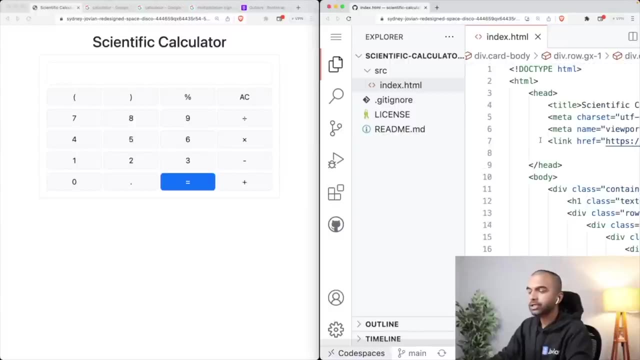 And that's going to now go and get added to our GitHub repository. Okay, perfect, Now we'll also see how to deploy this. So stay tuned till the end And, as I mentioned earlier, we'll also see how to do all of this. 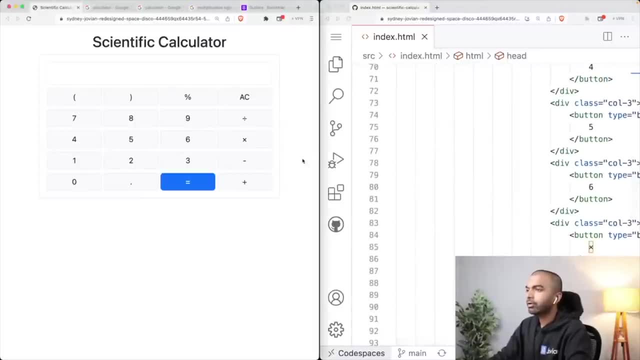 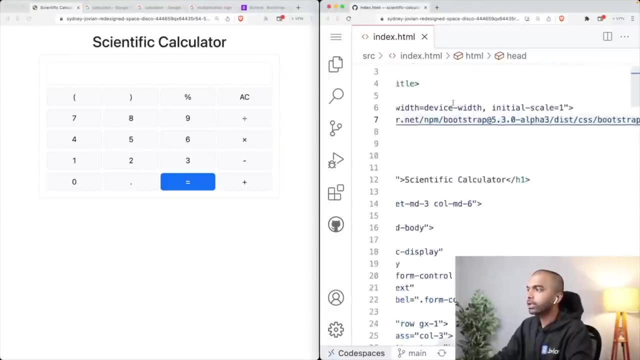 or most of it, using something like chargpt. Okay, now let us start adding the functionality for this. And to add the functionality for all of this, we are going to have to use some JavaScript, So I'm going to assume basic knowledge of JavaScript here. variables, data types. 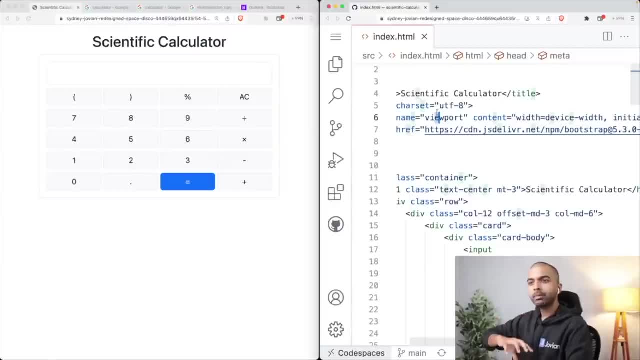 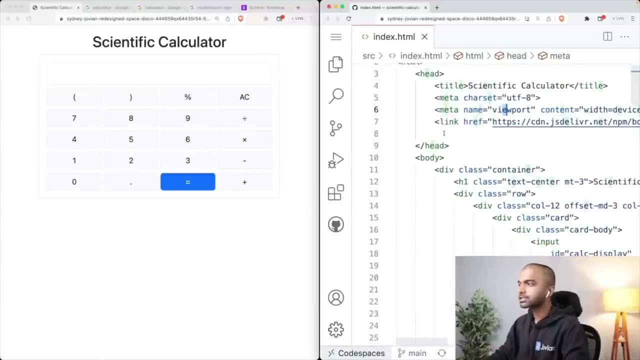 functions, And I'm going to show you how you can use JavaScript within an HTML page, And there are various ways to do it, But the simplest way to do it is by using a script tag, So you could, for example, go to this bottom of your body. 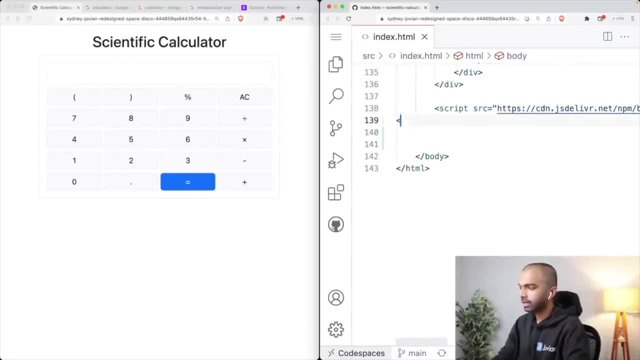 and add a script tag here. So I'm just going to go in here and add a script tag and you need a closing script tag as well. Okay, And you can also put in: yeah, I think that's it, And then now you can put in anything. 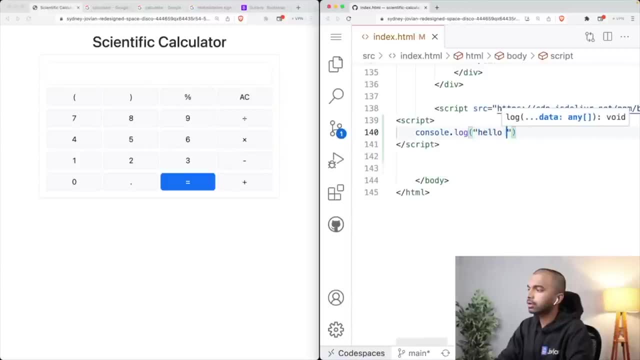 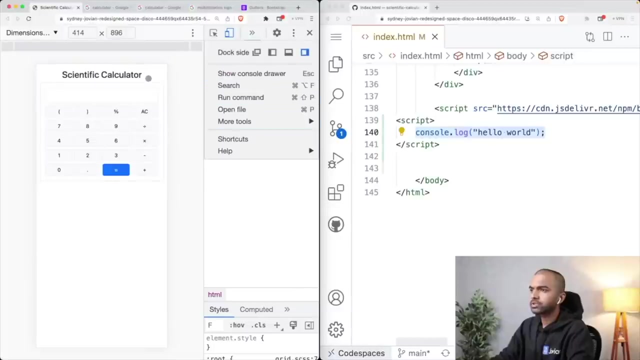 inside this So I could put, for example, consolelog: hello world, Okay, And now this. anything you put within the script tag is JavaScript code. So now you can actually check, you can inspect, Let me. yeah, So this is the mobile view. I think that's fine. 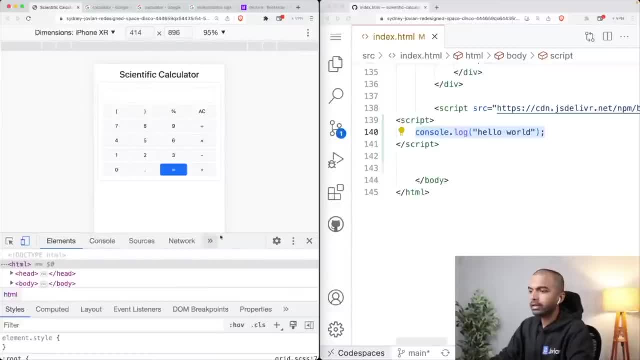 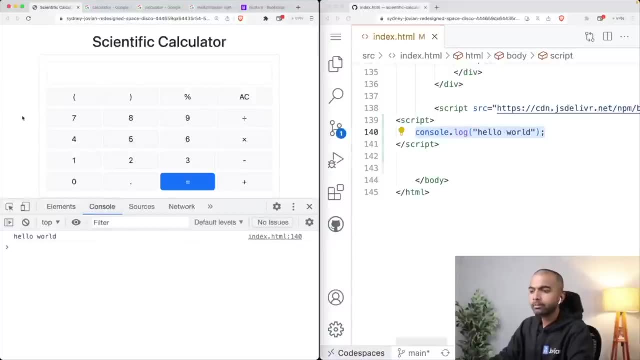 but let me just bring the doc down to the bottom and let me also turn off device mode for now. Yeah, So you can actually check the console tab here, Off the developer tools. You can always go go here from window developer tools or. 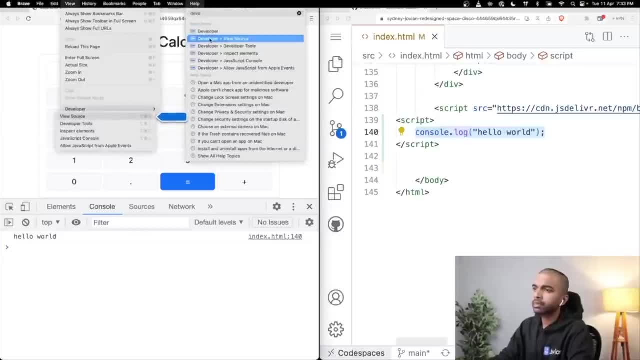 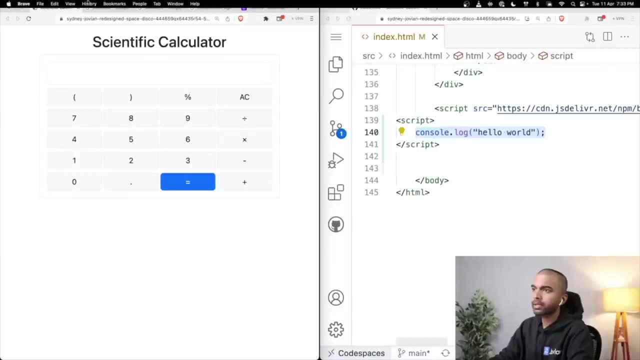 just type developer tools here from the okay. It's from the view tab. So view developer developer tools or JavaScript console. That's going to bring you to this page, So view developer JavaScript console. There's also a shortcut for it. You can see here that we typed consolelog. 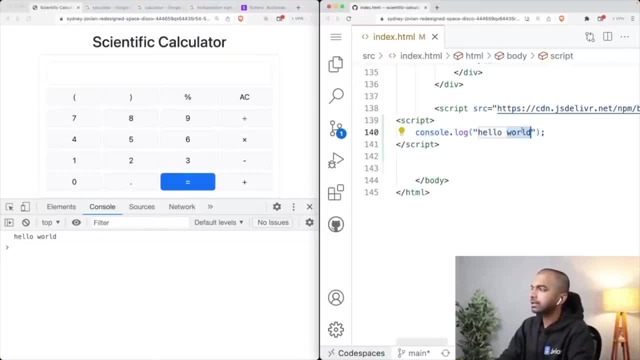 hello world and that printed hello world here Instead. if he had said hello Jovian, That would say hello Jovian. So this way, you can add JavaScript code within your HTML. Now, of course, we need a way to actually connect this JavaScript code with the buttons that we are. 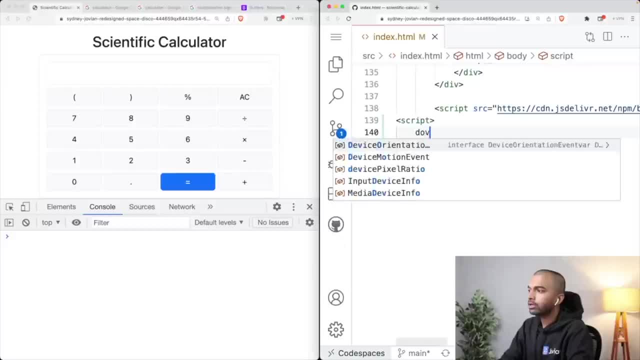 seeing on screen. So the first thing we'll do is we're going to say: document dot on ready, Yeah, something like that. So, uh, what do you? what we want to do is we want to make sure that we run the JavaScript only after the entire document has been run. So we're going to run the JavaScript only. 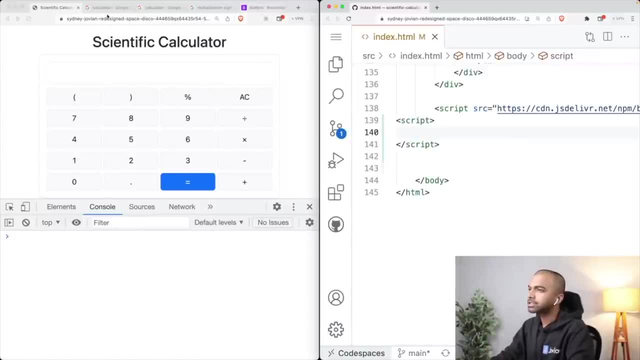 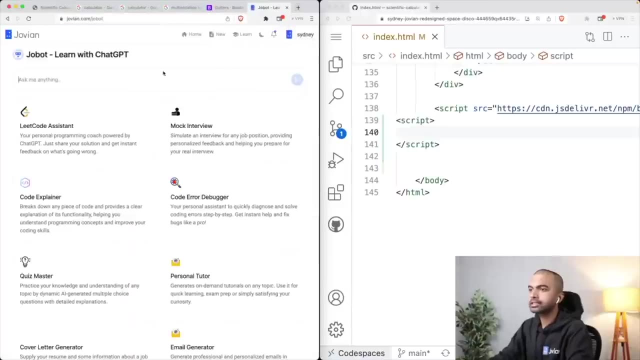 after the entire document has been run. So we're going to run the JavaScript only after the entire document has loaded up properly. So I'm just going to go in maybe and ask this on Jobot, our chat GPT powered chat assistant. So let's see how to how to run some JavaScript code. 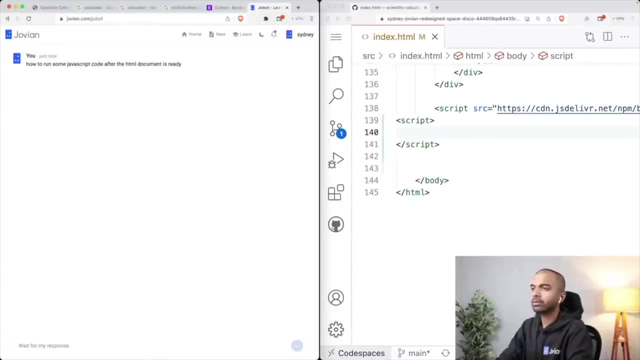 after the HTML document is ready. Okay, And it's going to tell me some explanation which you should read. Absolutely Okay. So basically, what it's telling me is that if you want to run some JavaScript code, if you want to interact with an HTML page, after the HTML page. 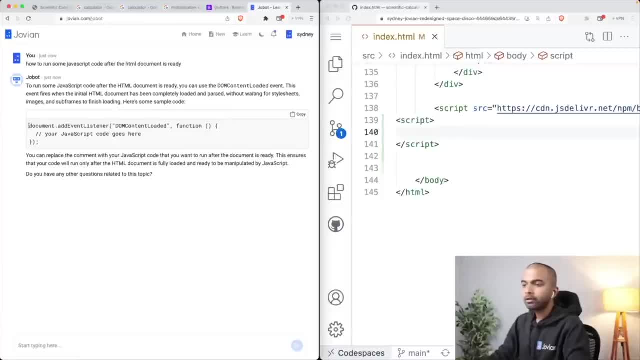 is loaded up properly, then you need to put in your JavaScript code inside this piece of code. So basically what we are saying here, I'm just going to first come in and paste it in here. So basically what we are saying here is that to the document, which is the entire HTML document. 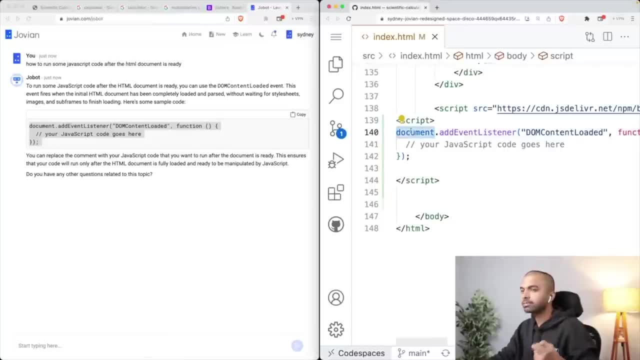 and this is a predefined variable. in JavaScript there's a bunch of predefined variables like window, document, et cetera. So to the document we are adding an event listener, Which means when this event occurs, we want to do something with it. What is the event that we're? 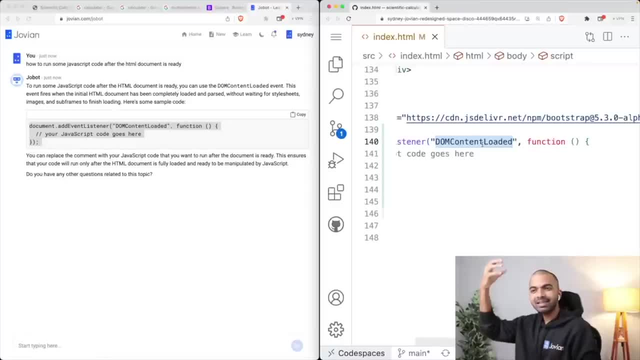 looking for? We are looking for the event DOM content loaded, which means that the entire page, the HTML, the CSS, et cetera, the entire page has been loaded in by the browser. And when that event or when the entire content has been loaded, then we are asking the browser to fire this. 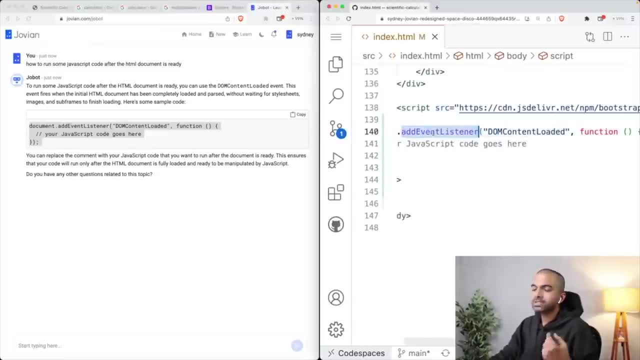 JavaScript function. So you can see that we've provided two things to add event listener, which is a function or a method, inside document. We've added two things. We said when the event DOM content loaded is fired- which means when the entire content is loaded- then call this function. 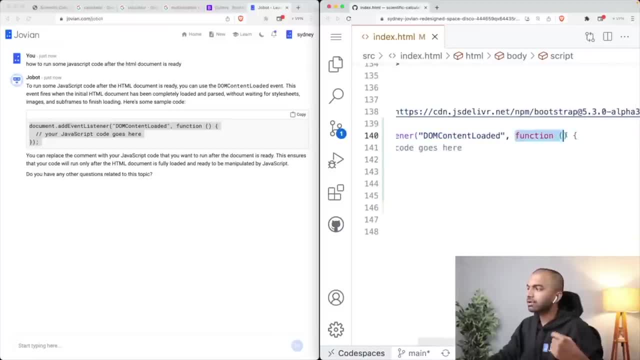 inside. call this function or call the code inside this function. Okay, And that's why we're providing it as a function, because the function can be invoked when the event occurs and not. we don't want to run this code immediately, We want to run it only after the page is ready. Okay. 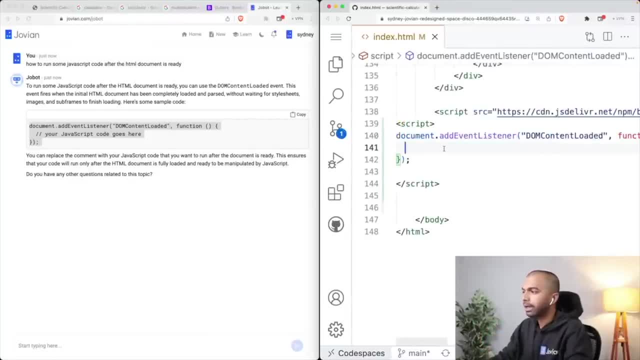 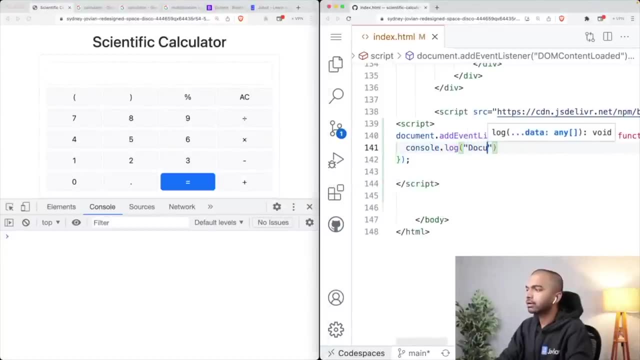 So that's how you add some JavaScript code into an HTML page. We want to do here. I guess first thing to do is maybe just once again add that console log saying that document is ready and let's just see. then you can see here Now the 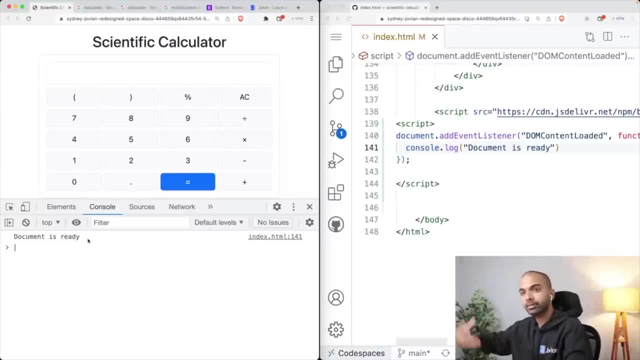 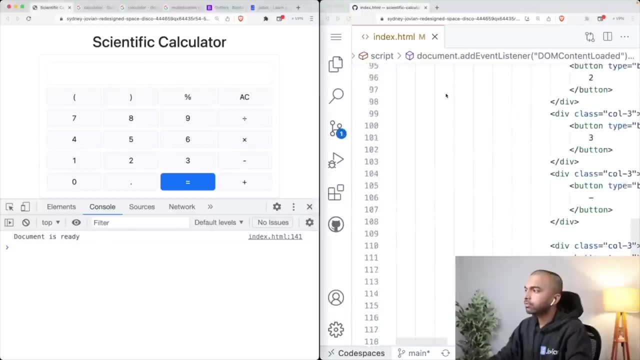 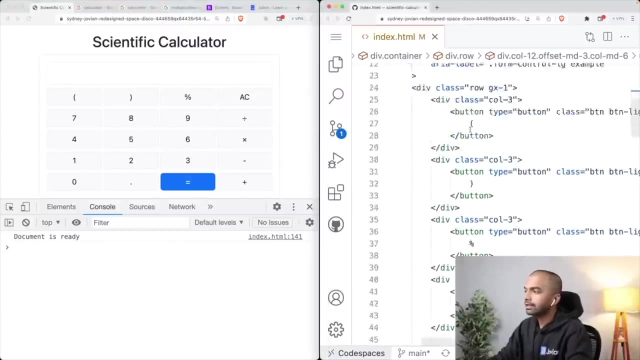 same thing is printed. document is ready, but of course, it is printed after the browser has loaded the entire content. Okay, Now let's get, remember, this input over here. we have given it an input. We have given it an ID calc display. Okay, We've given an ID calc display, So let's first get this. 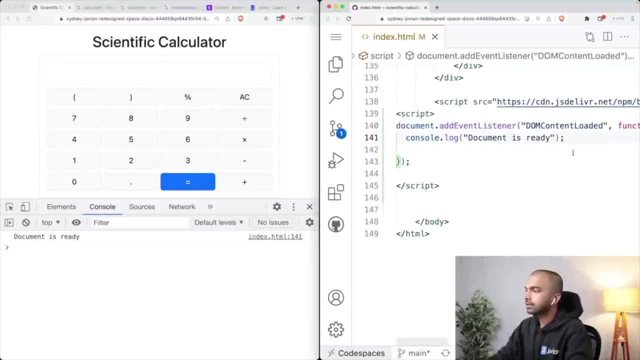 input. Let's get a hang of this input. Let's get a hang of this input. Let's get a hang of this input. So let's, um, let's call it display. So let me say: const display equals document, dot get. 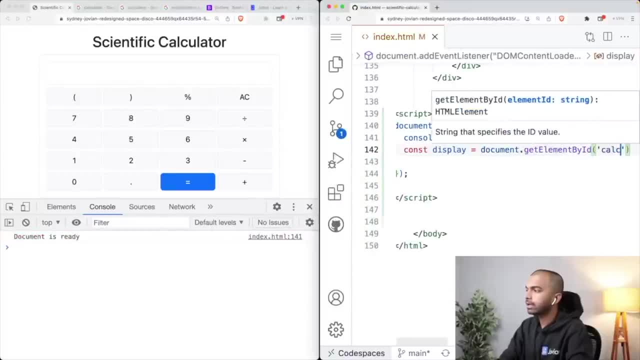 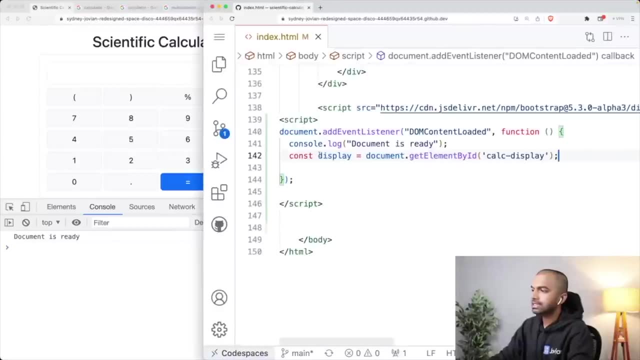 element by ID: calc display. Okay, So what we're doing here is we're saying that we want to get the HTML element which has the ID calc display and document dot get. get element by ID is the function you use to do that. We want to get the calc display. 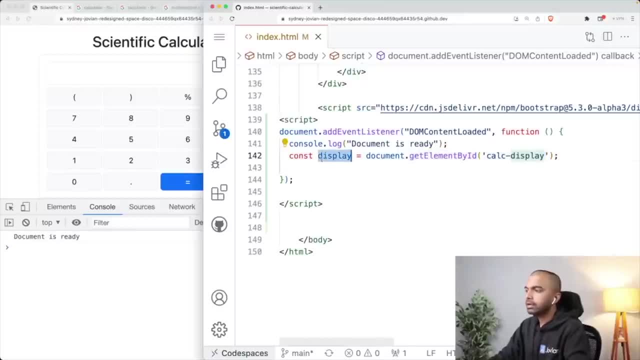 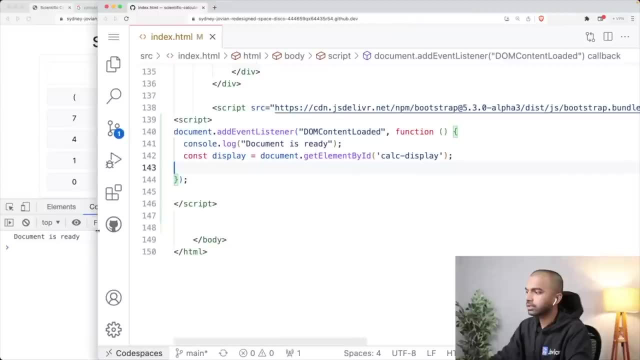 and we want to store it in the variable display. Okay, And now we can just do console dot log display, for example. Okay, Let me fix the tab size over here. Looks like it's just adding a bunch of spaces that I don't need. indeed, using spaces and two spaces. Yeah, All right, I'm good. 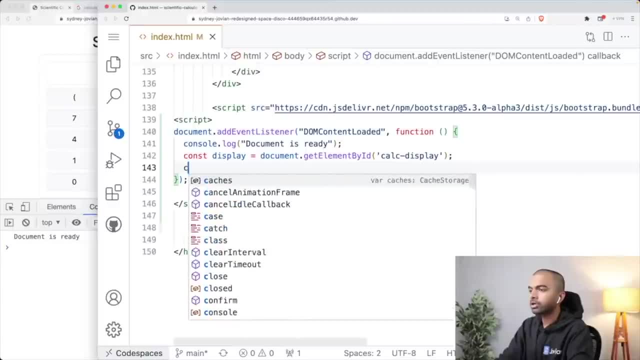 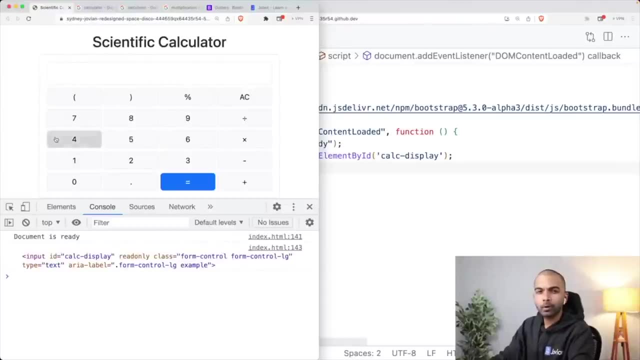 So now we have this knowledge through console dot log display. Okay, And now you can see here that as soon as the document loads, our job script code is searching for the element with the ID calc display and it is simply printing it here. 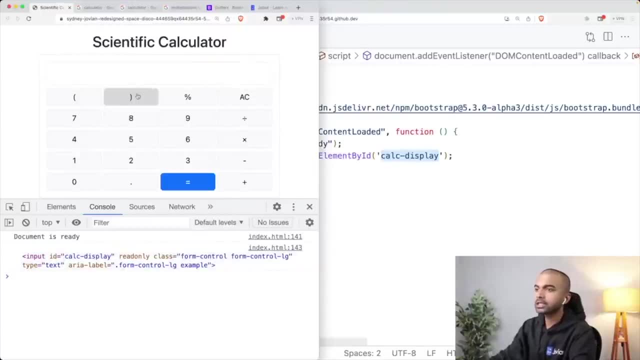 in the console And you can see when I hover over it. it actually shows me on the screen right over here that the input box is what, um, this element is referring to. Okay, So now we've gotten a hold of our input box. Now let's try to get a hold of all these buttons. Okay, How do we get all? 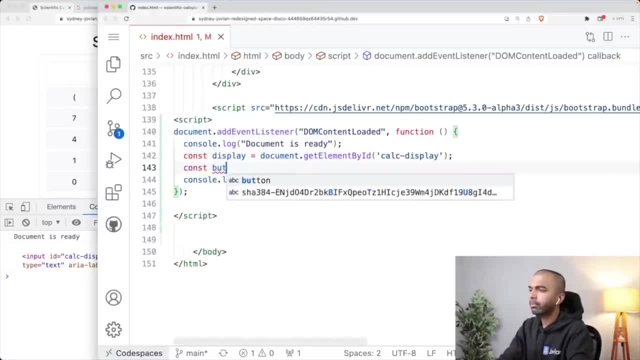 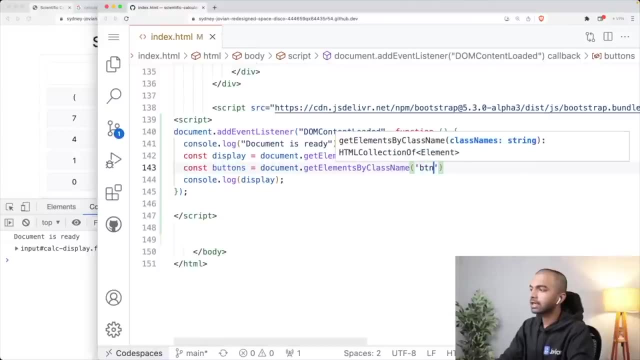 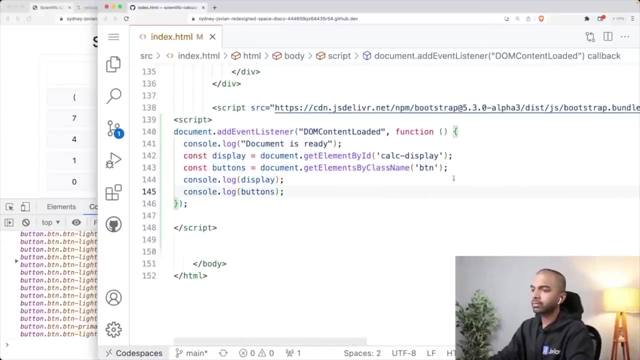 these buttons. Well, let's see const buttons. equals document dot. get element By class name, And I think all the buttons have the class name BTN and I can say console dot, log buttons. Okay, great, So you can see here that each button has. 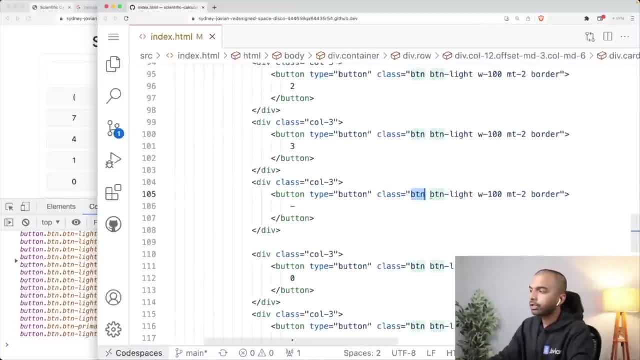 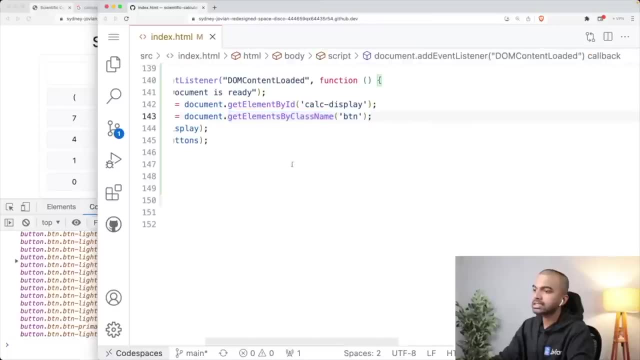 a class BTN, All right. So we have gotten a hang of all the buttons with all the elements with the class BTN simply by saying document dot. get elements by class name- BTN. Okay, And you can see here that we've printed them out and it says that it's an HTML collection. So we're going to. 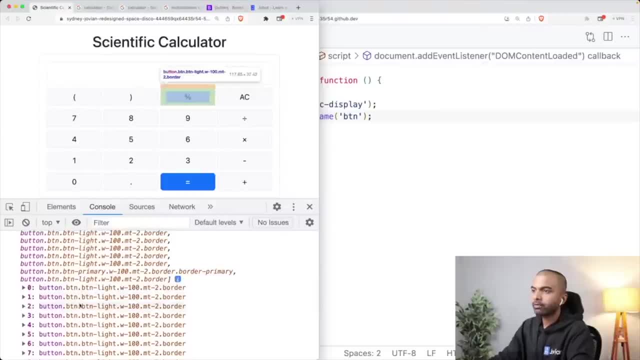 have an HTML collection of 20 buttons And each button- as I hover over it you can see that shows me that specific button. So that's the first thing you need to understand whenever you're writing some JavaScript code to add interactivity- interactivity into an HTML code, you can. 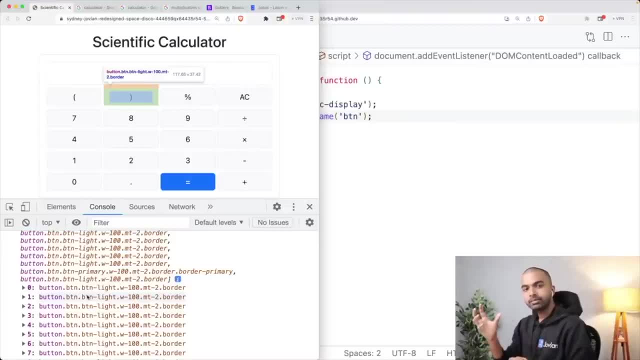 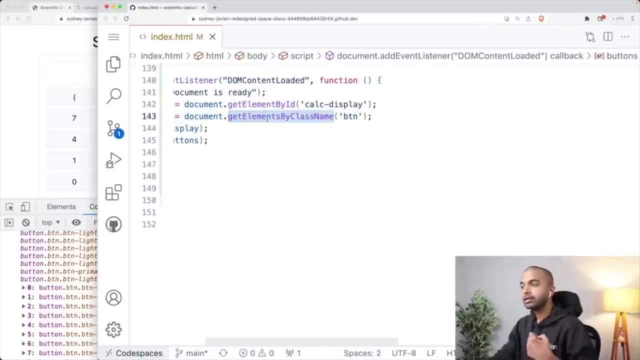 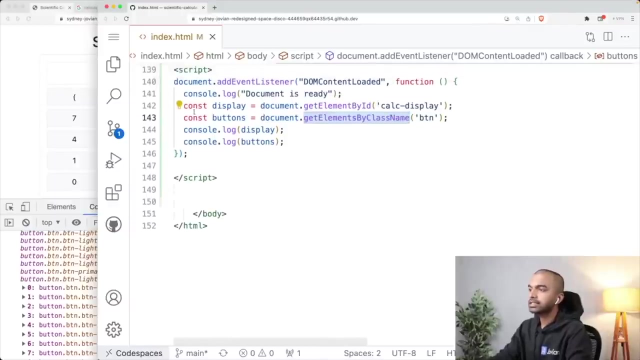 simply select some HTML node using things like document by dot, get element by ID, or you can get element by class name, or you can get element by tag name. there are a bunch of ways and you can use it to add those HTML elements or references to those HTML elements in these, in variables of. 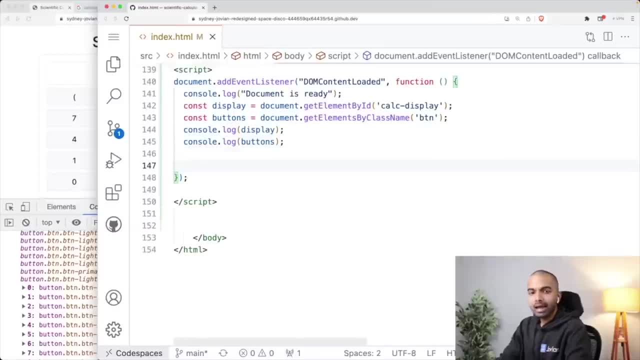 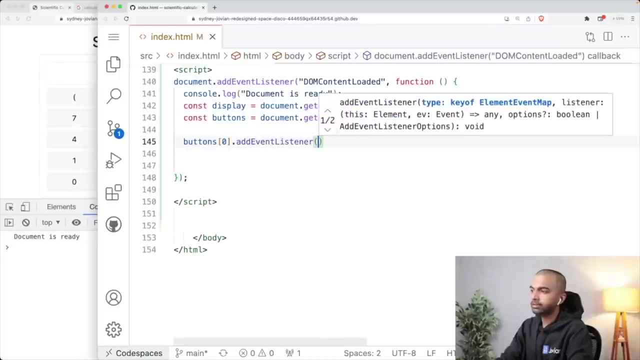 your choice. Okay, All right. next up Now, let us maybe try to add a click handler to one of the buttons. Let's do something when a button is clicked, So let's say buttons zero, and that should simply pick the first button. dot- add event listener. So again, now I'm adding an event. 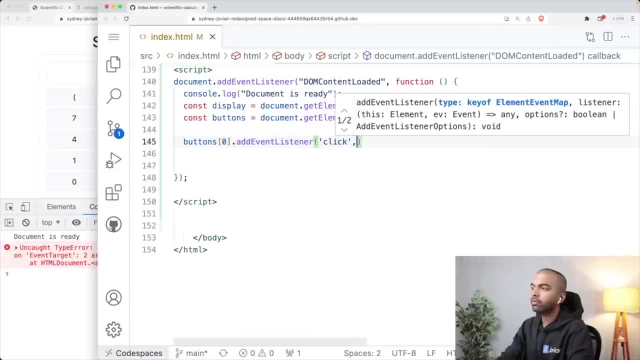 listener to the button. And what event do I listen for? a want to listen for. I want to listen for the click. so i'm saying when the button is clicked i want to run a function. so i have to provide the function that is going to get executed when the button is clicked. okay, so the function that 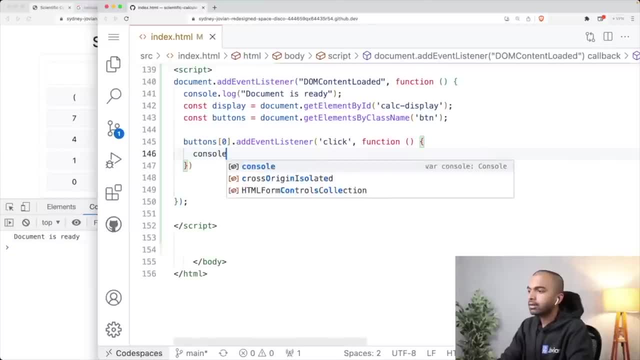 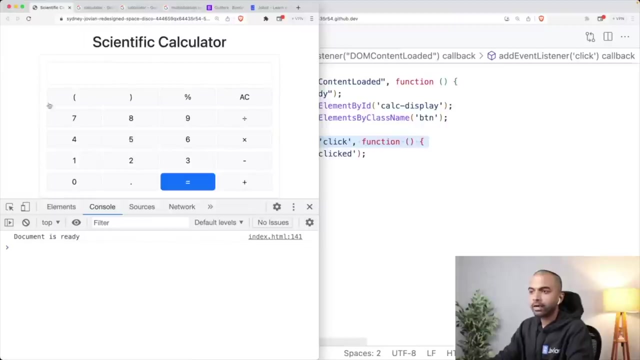 gets executed when the button is clicked. for now, i'm just simply going to say: consolelog: first button clicked, all right, and now you can see that i have this event listener attached to my first button and nothing happened so far. you, we are not printing. first button click and let's 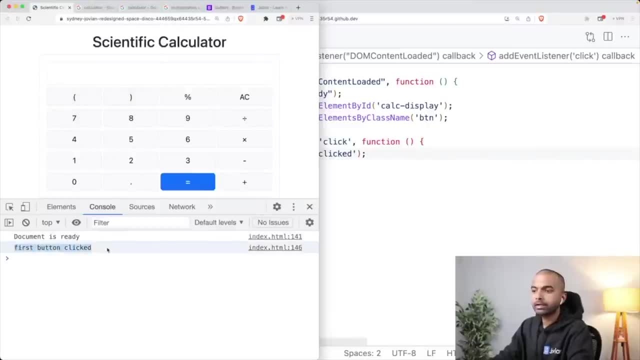 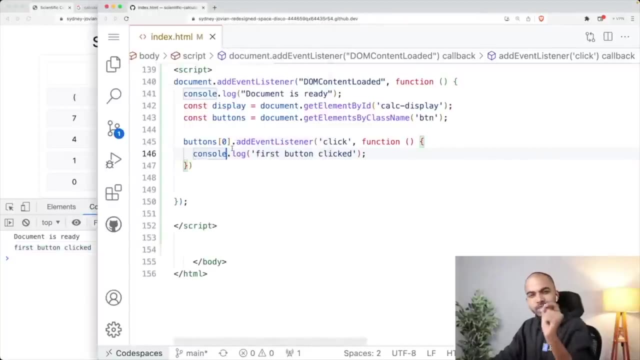 say, i click the first button, you are going to see printed your first button clicked. so that is the next thing you want to understand: that you can add event listeners or click handlers to specific dom nodes. in this case it's a button and you do that using add event listener and you can do that not. 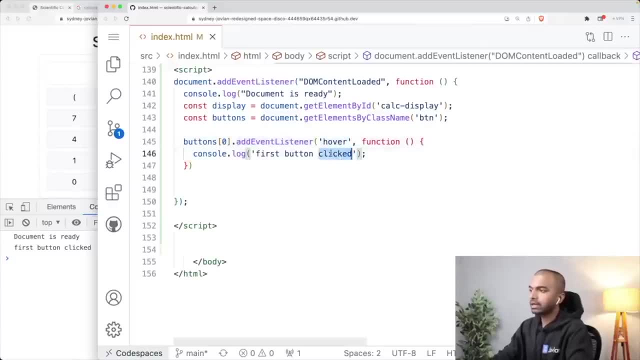 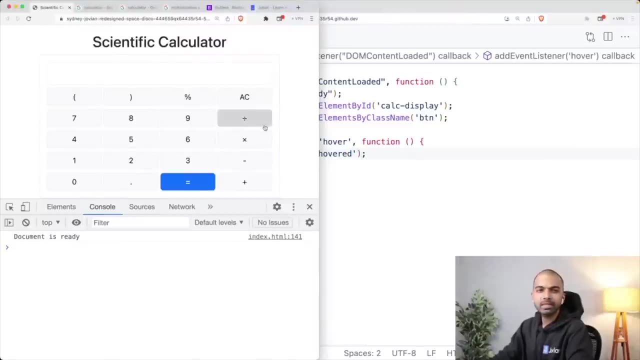 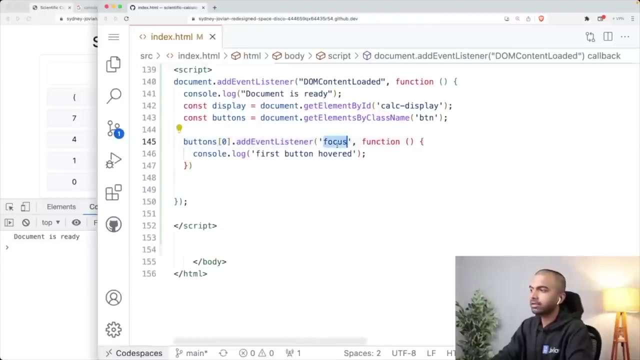 just on click. but you can also do hover, and let's say i could just then print out: first button hovered. and this time what happens is when I simply, Well, maybe not hover, maybe it's some other event, I don't know, like focus, I don't know. Well, there's probably some event out there, But yeah for. 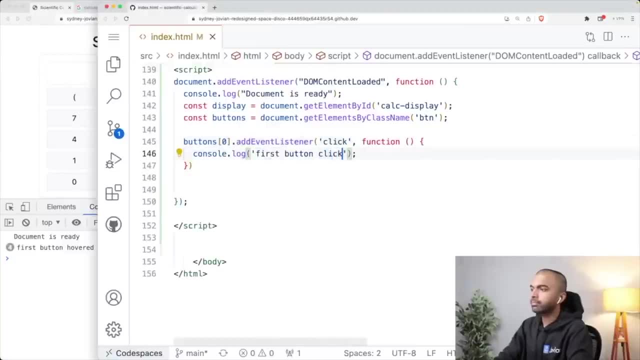 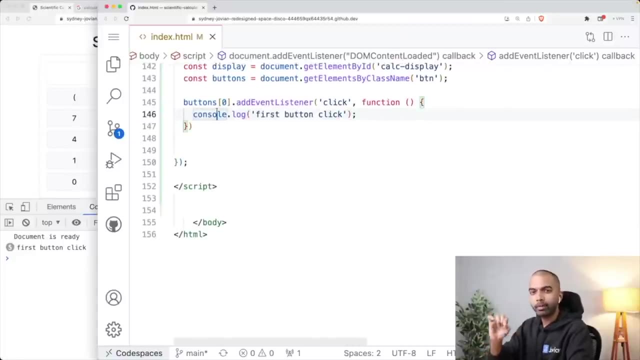 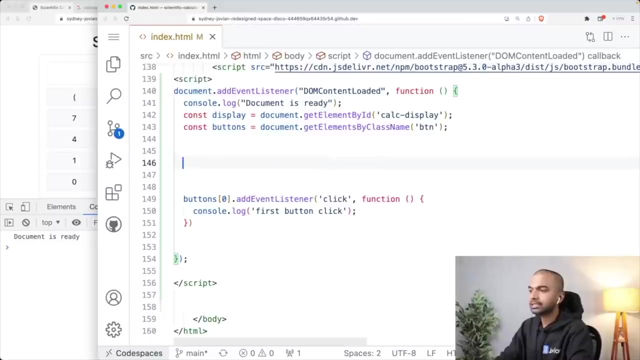 click. you can simply get some something printed out on clicking. Okay, Perfect. So now we've added a click listener to one of the buttons, But ideally we want to add click listeners to all of the buttons at once, or individual click listeners to all of the buttons. How do we do? 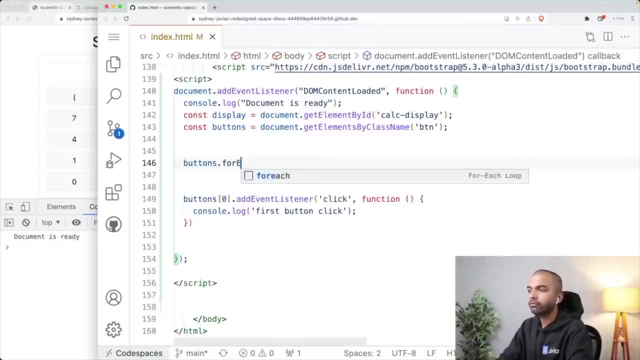 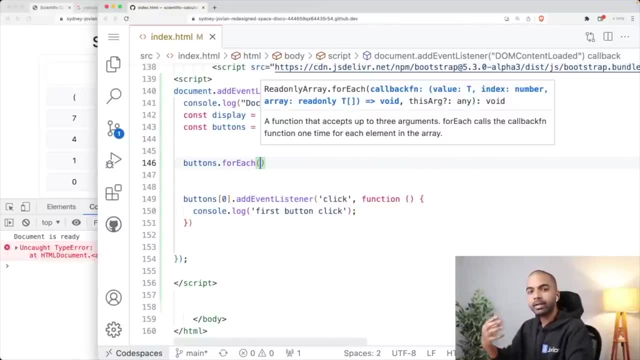 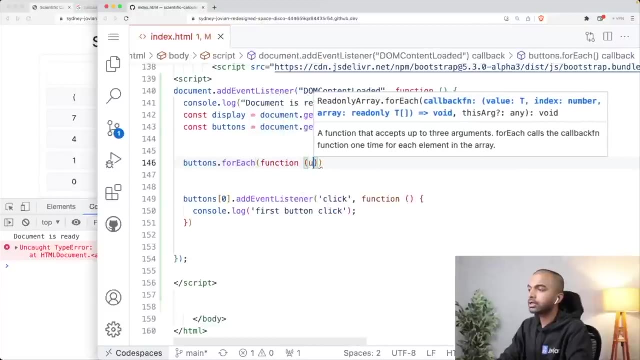 that. Well, we can do something like this. we can say buttons dot for each, So for each is a way for you to do something for every element in a array, in a JavaScript array, Okay, So what you can do is you can now provide a function to for each, okay, which is going to take each individual. 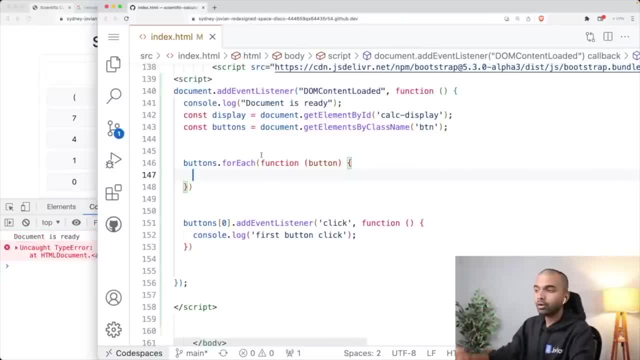 button And it is going to operate that on the individual button. So the button now is going to refer to each button button one by one. And now I can say: console dot, log button clicked And from this button maybe I can get the text of that button. So button dot- inner text. So if you want to get, 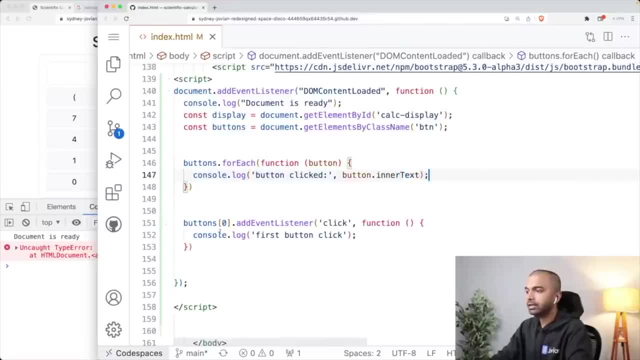 the text inside an HTML element, then you do that simply by simply by calling dot inner text. Okay, that's a property. Let's see. Maybe it's for each without a Yeah like that. Okay, So let's turn that into get elements by. I could just use a for loop here. I think that would be simpler So. 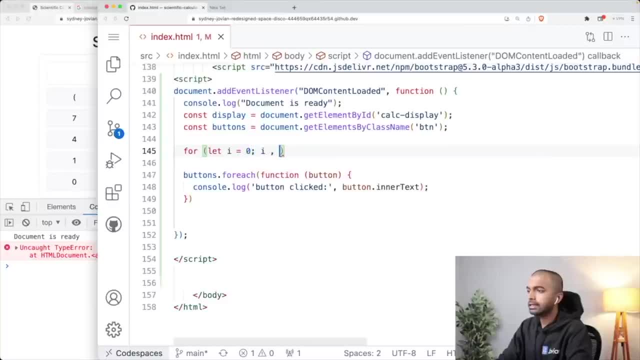 for let i equals zero, i less than buttons. dot length I plus plus a for each would have been nice, but looks like there are some problems when you're working with an HTML collection. you probably can't do for each or something But button. so 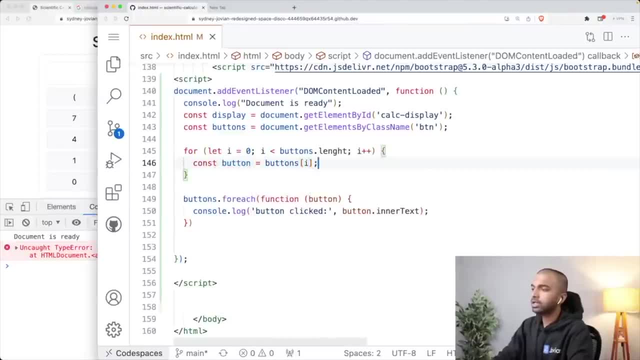 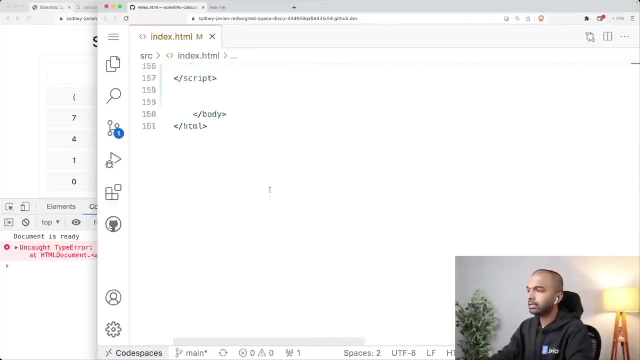 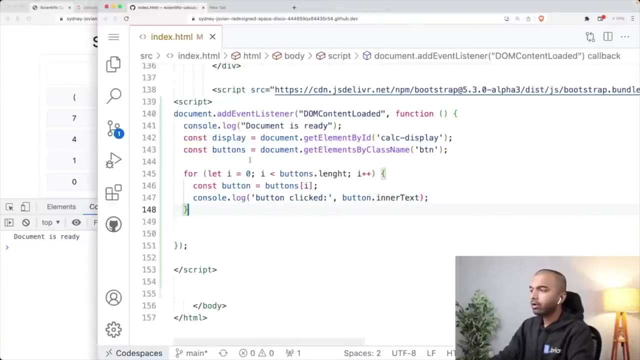 const button equals buttons i. So what I'm doing here is I'm looping over the list of buttons and I'm getting each button And then I'm saying button clicked button dot inner text. Okay, Alright. so now what we've done is, for each button, we are simply going to log. 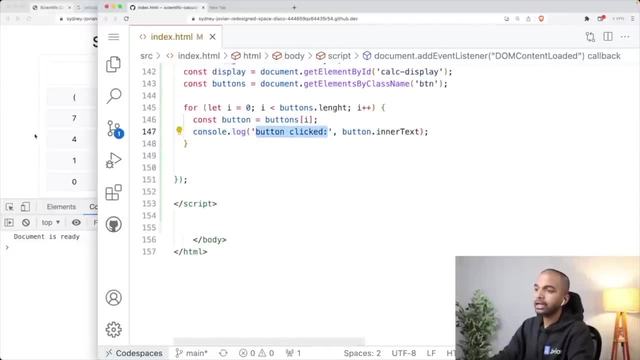 that the button was clicked when the button is text and we're going to log the inner text of that button. So I need to add that actual click listener. So I need to say button dot, add event, listener, click. of course we want to do the console log only when the button is clicked. 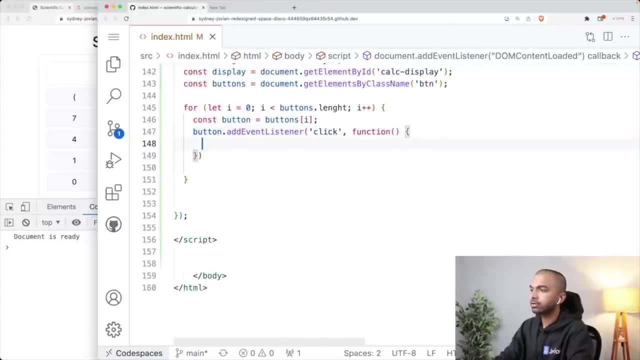 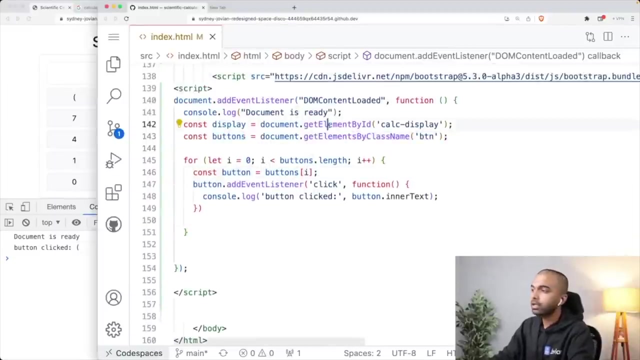 and not always. So. let's add this console log only when the button is clicked. Okay, Alright. well, let's see what's a, le, n, g, th. that should fix it. Yeah, Okay, so now you can see here. all we've done is gotten a list of buttons using get elements by class name. 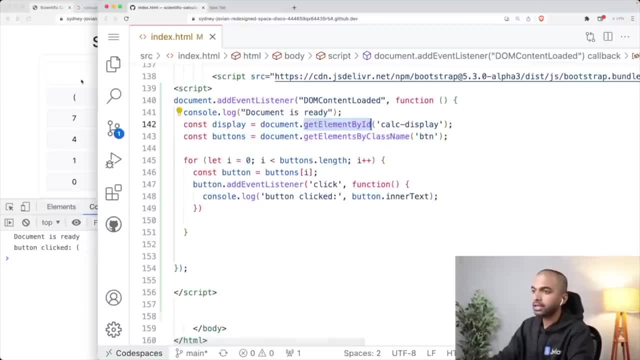 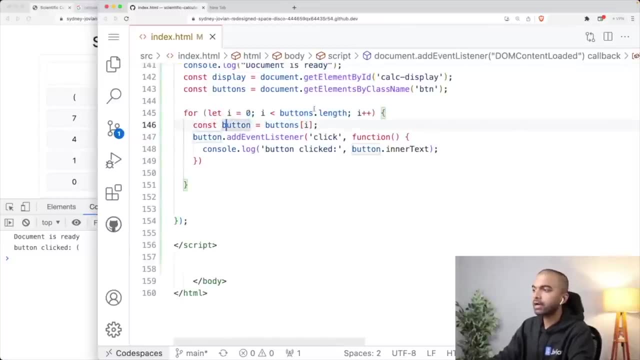 gotten a list of the actual doc, the actual display, input display using get, element by ID. And now we are looping over the buttons. using this for loop, we are saying i equals zero, i less than buttons, dot length, i plus, plus, and we're getting each button as buttons i and then. 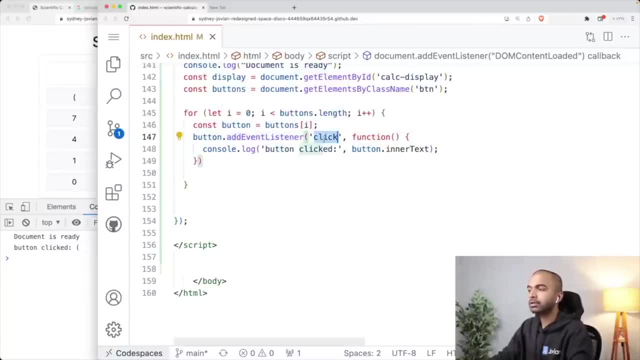 we're adding a click list, So we're getting each button as buttons i and then we're adding a click listener- event listener- to each button And on the event click we want to invoke this function. Okay, the function that that's going to get invoked is simply going to say: console dot log. 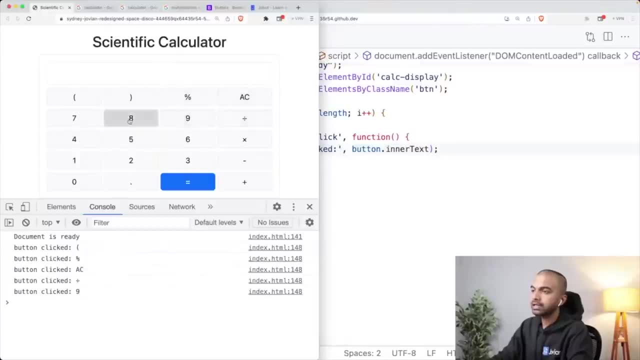 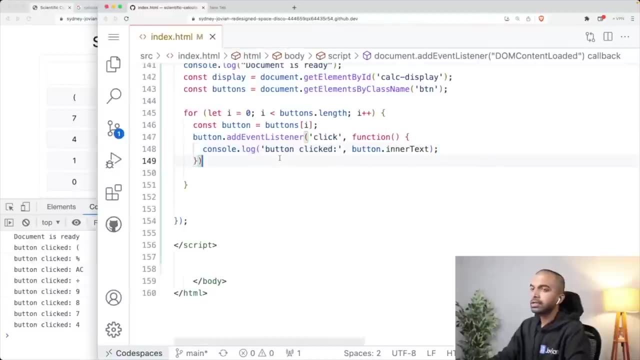 button clicked. And now, when I click on a button, you can see that each time we simply print which button was clicked: button click percentage, button click 987, etc. Okay, so it's a bit of work to hook up JavaScript code with some of the event handlers for specific DOM nodes, for specific nodes on the 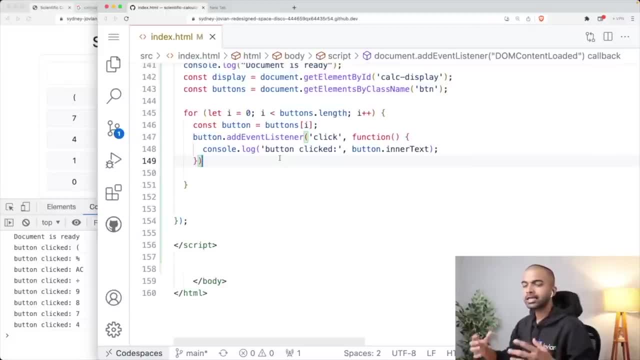 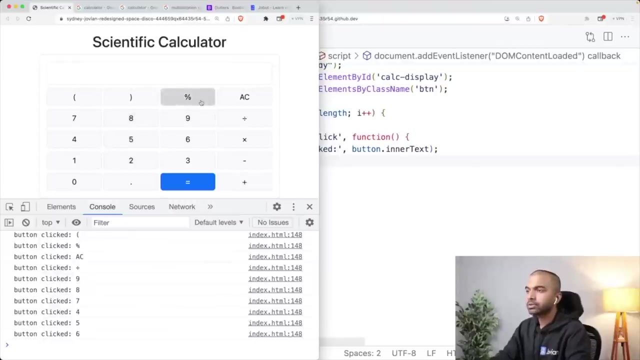 HTML page. That's why a lot of people use frameworks or libraries like jQuery, react, etc. But this is just raw JavaScript. we are simply picking up the button, we are attaching an event listener to it, And this is what it's doing. Okay, Now, of course, what we want to do instead is not actually use. 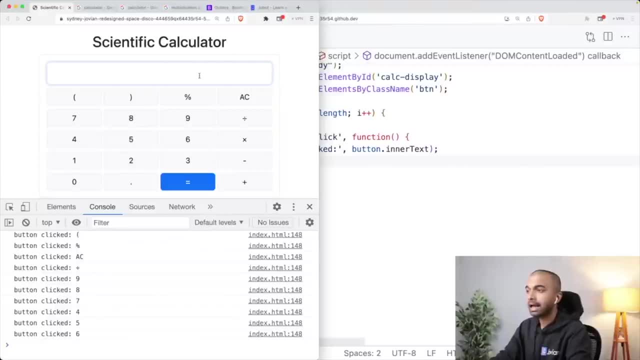 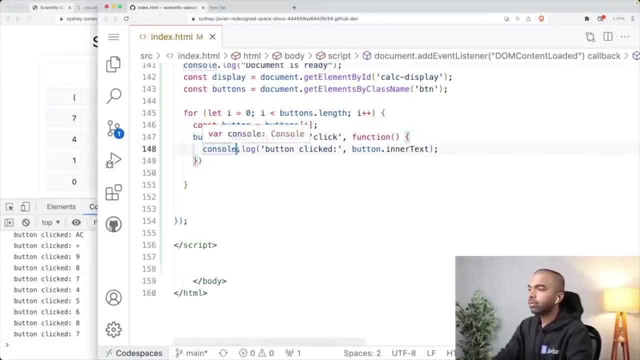 the console logged event but simply add that here in, add that information here. For example, if I type seven, I just want seven to be added here, Okay, So here's what we can do about that. So let's say in this button: let's do this. let us first keep track of the current value of the input. 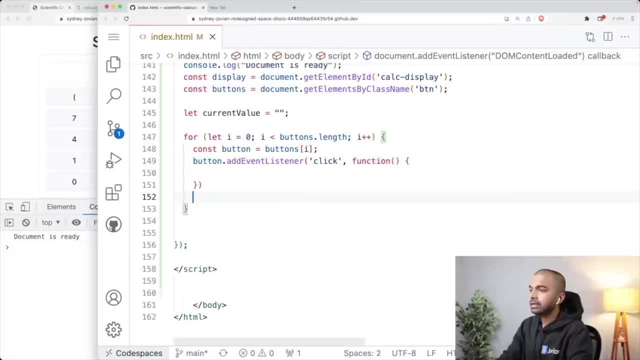 in a variable called current value. Okay, so let's do that And let us say const value. So this is the value that is present inside the button. is simply button dot inner text. Okay, And now I can say: current value plus equals value. Okay, so we have adding, we're. 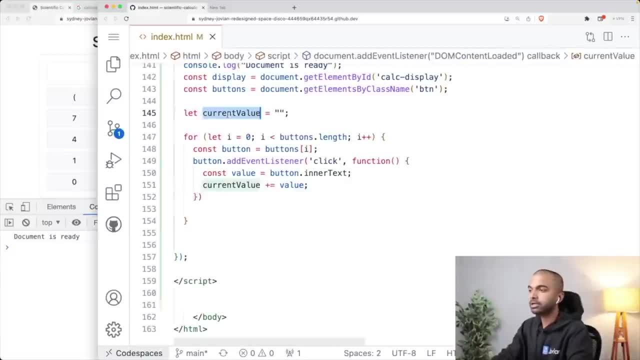 adding the inner text of the button to the variable current value, which we have here, And then we can say current value. Then we can. we have the display here, So we can say display dot value. Remember display, this is simply the input box over here. So we can say display dot value. 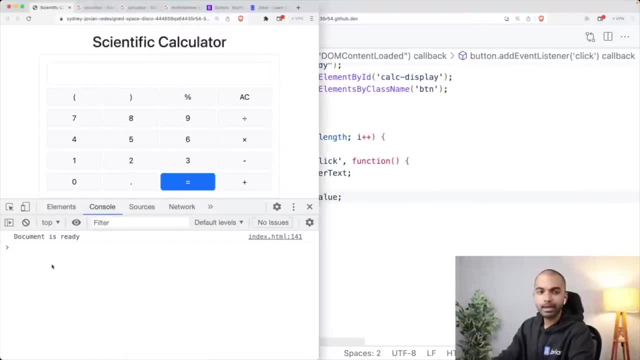 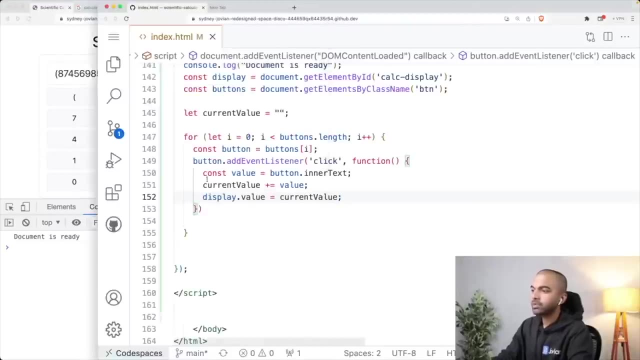 equals current value. All right, so let's try that out. Okay, so you can start to see here what's happening As soon as we. so what we're doing is we're creating this variable current value. it contains the empty string right now. 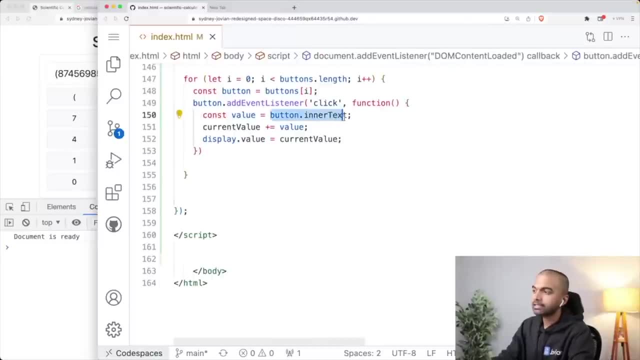 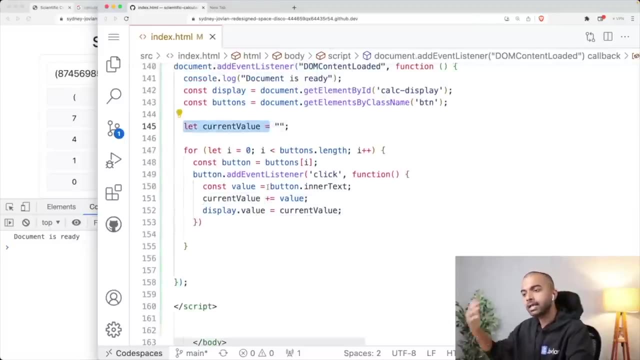 But what we're then doing is, when a button is clicked, we're getting the inner text of the button, adding it to the current value. So the current value now contains the empty string plus the value from that button, plus the value from the next button that clicked, and so on. 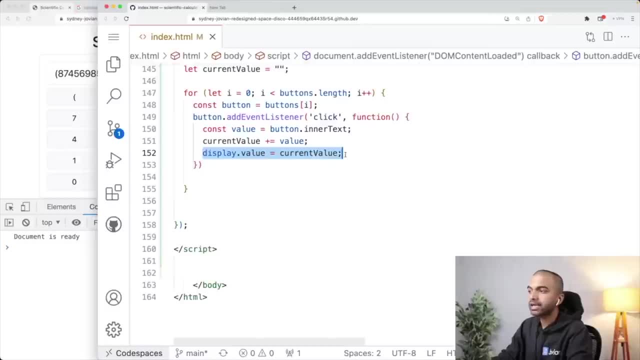 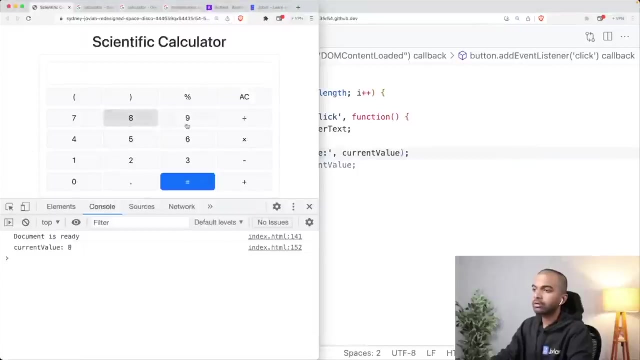 And then one very important thing we're also doing is we're also setting the value of the input box box to current value. If we didn't have this, then current value would keep changing. So we could just log current value over here. Okay, we could just log current value over here And you. 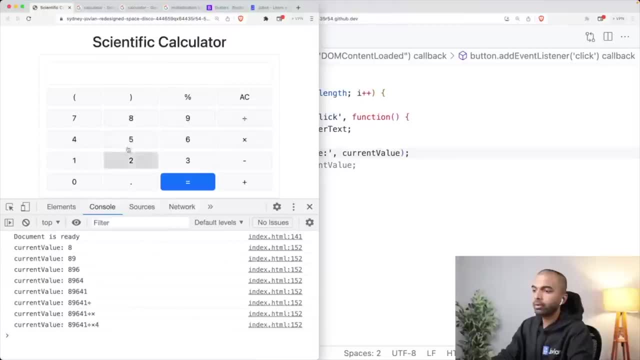 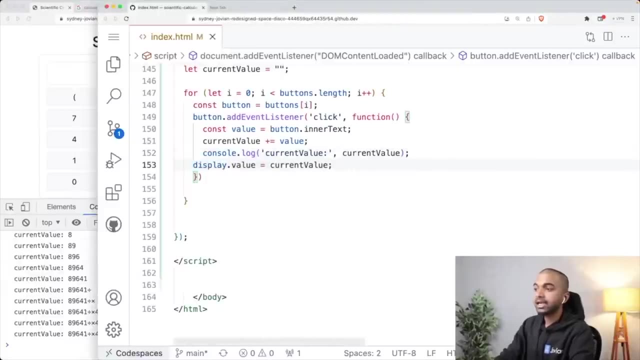 can see current value is changing to whatever I set it to, But this is not changing. there's nothing is getting added here, And that is where you can actually set the value of the value inside an input field And you can change the text inside a particular div And you can do all sorts of. 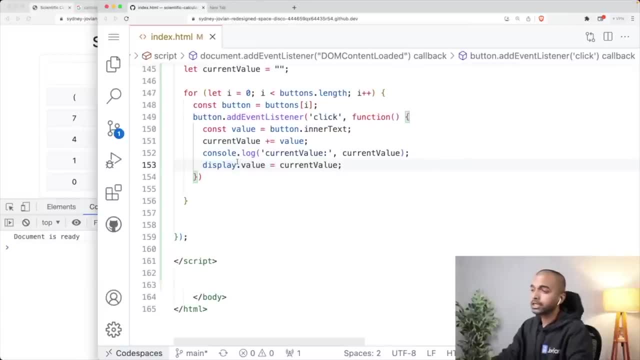 things. So, basically, you can modify the content on the page using display dot value or display dot inner text or whatever you want to want to use for it, And you can set it to some value that's coming from a JavaScript variable, or you can just set it to something manually. Okay, so that's. 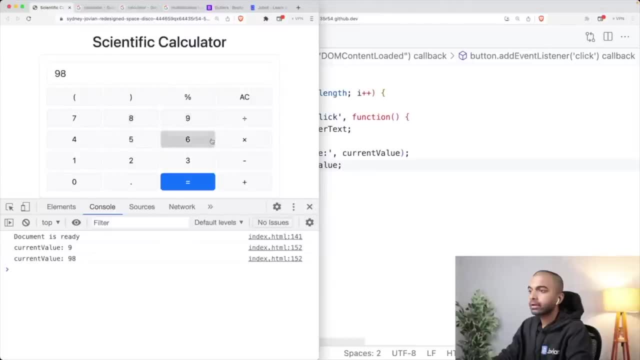 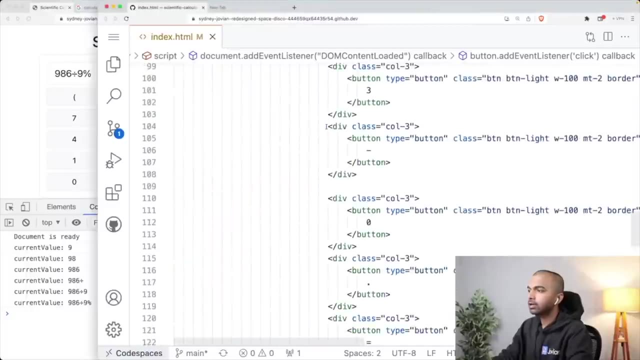 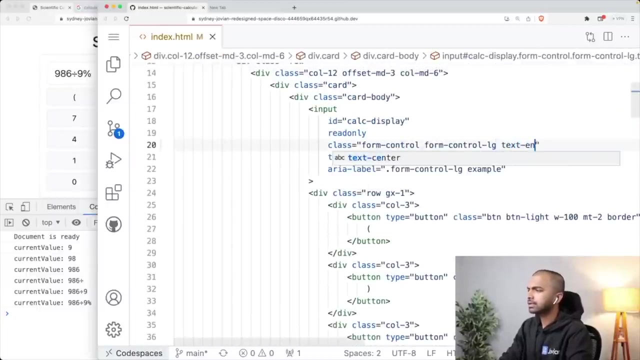 great. So now we have this functionality And I think one thing we can do is maybe bring it to the right instead of the left. So I'm just going to come back in here into my text, into my HTML code, And I'm just going to say for this input text end. And I believe 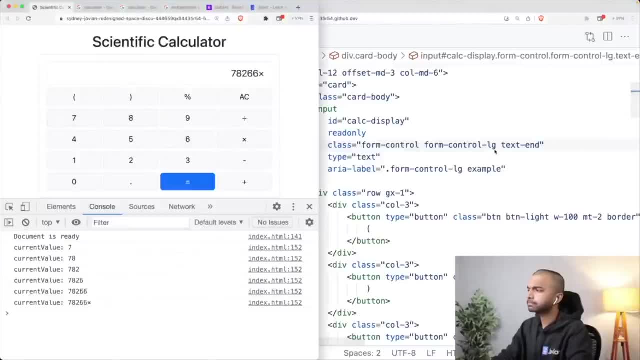 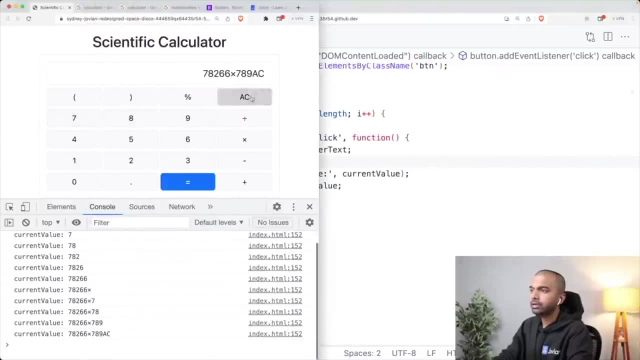 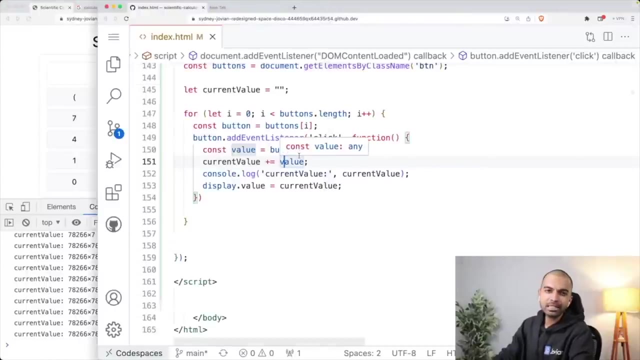 that simply going to orient the text at the end for it, And that's looking good, Okay, So now we're able to actually capture this value, But of course, we are not actually working with the equal to yet. So we need to handle equal to, we need to handle AC. let's start with AC. 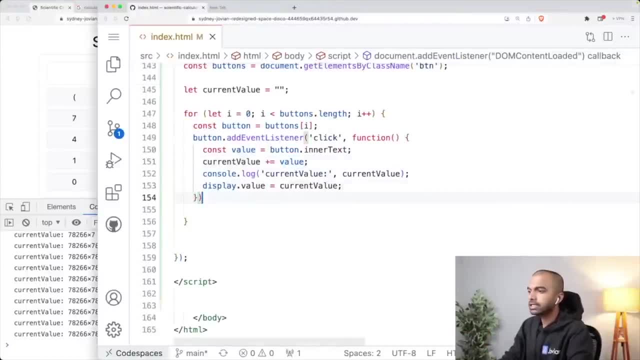 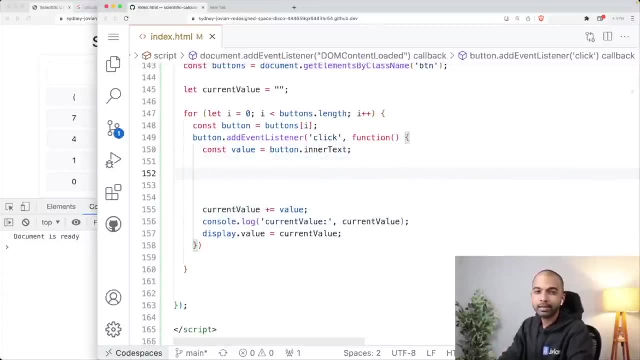 AC simply going to clear the entire thing. So let's start with AC. So what we can do here is we can actually do an, if else, on the value of the button text. So, based on the button that was clicked, we need to do a simple, we need to maybe run a separate piece of. 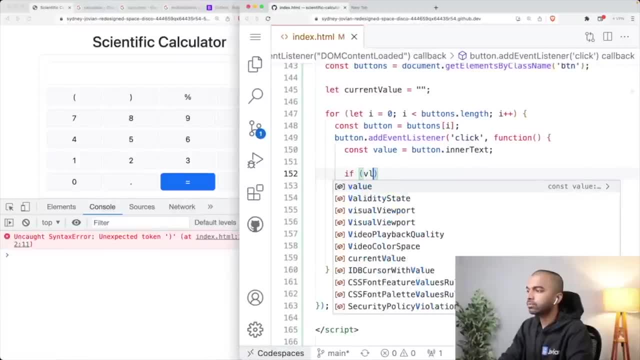 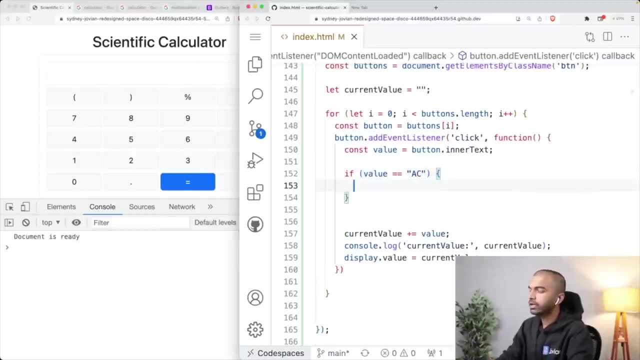 logic. So I'm going to say: if value, which is the button that was clicked, equals- and I'm just comparing here, that's why I'm using the double equal to equals AC- then we want to do something else. Otherwise we want to do something else, right? So else we want to do this. So let's get. 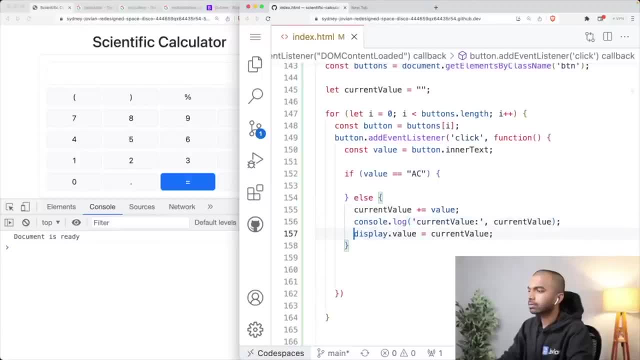 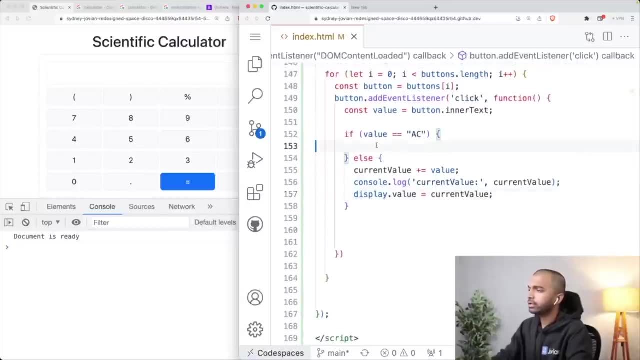 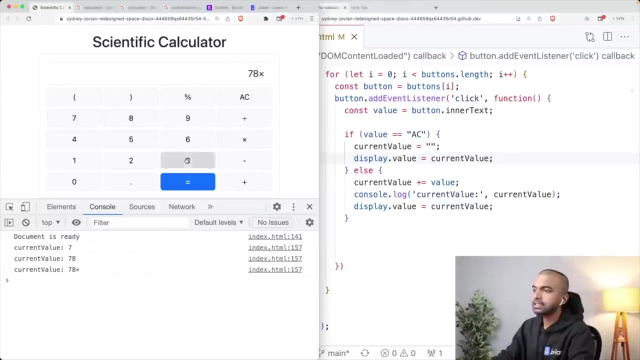 this into else. Okay, let's get this into else over here And let us now go in here and let us set the current value simply to empty. And again, let's just set display dot value equals current value. Okay, so now we've implemented the functionality for the AC button. 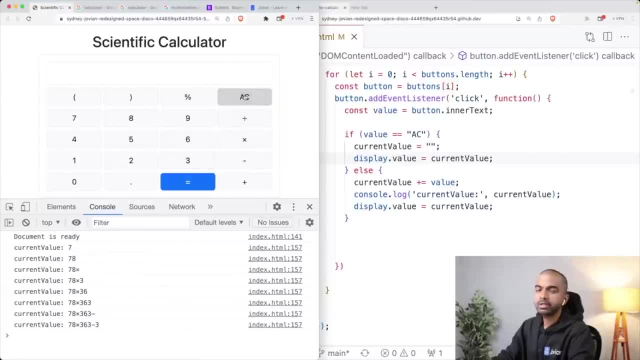 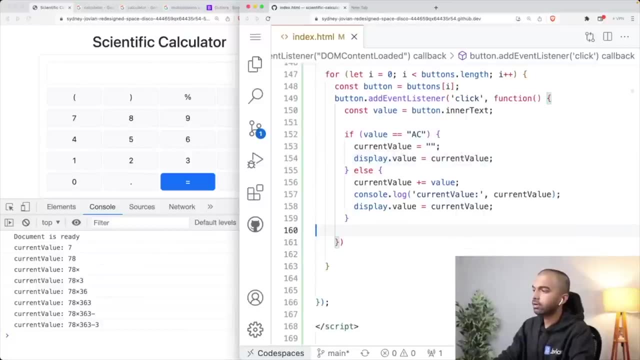 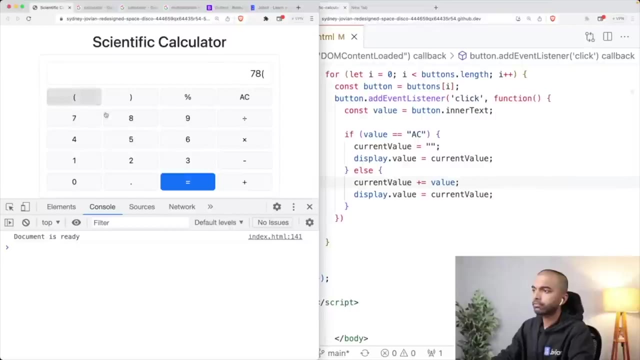 So let's say minus three, and when I press AC, you can see that simply clear, clearing the current value because its value is AC and it is setting the display value to the current value. Okay, so now I am, my things are looking pretty good. So now we are working. now this is working, Of course, brackets and all. 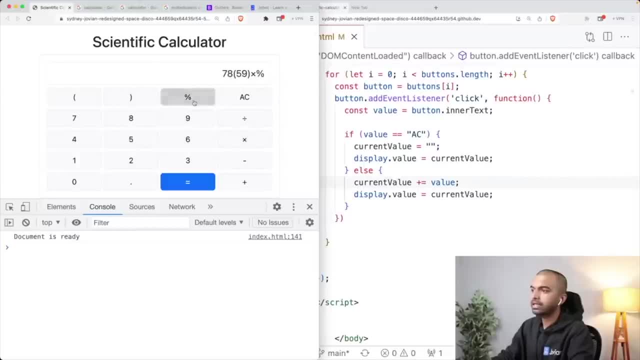 are also working. These may not be valid, valid expressions, But nevertheless, these expressions are working. The next thing we need to do is actually evaluate these. So when equal to is clicked, we don't want to insert an equal to. we actually want to evaluate these And for this, 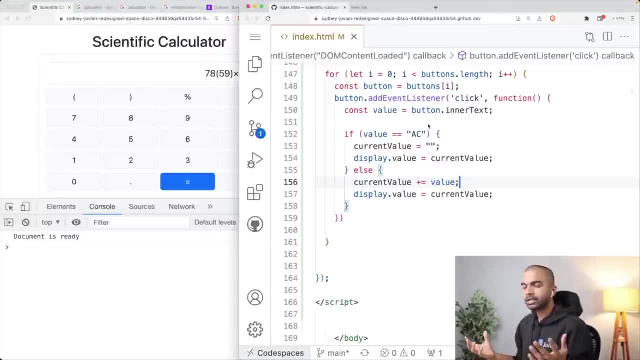 we're going to use a shortcut here. Normally, something, something like Google, would actually do a proper if else condition. they would parse the string and they would have some logic to evaluate it, or maybe they would send it to a server and evaluate it and get the result here. But we're just going to use a shortcut. 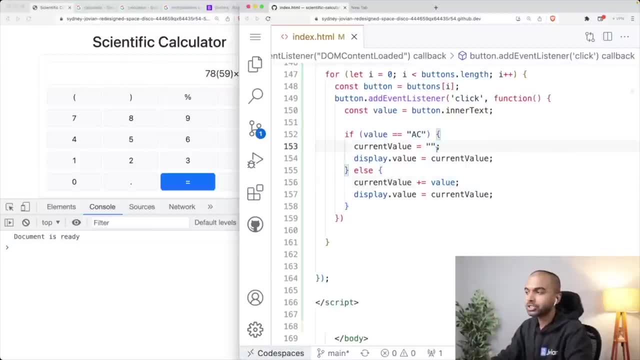 which is not safe to use in a production application. So I just want to tell you that. But here's what we're going to do. Let's put another else if over here. So let's say else if and after else if. let me just. 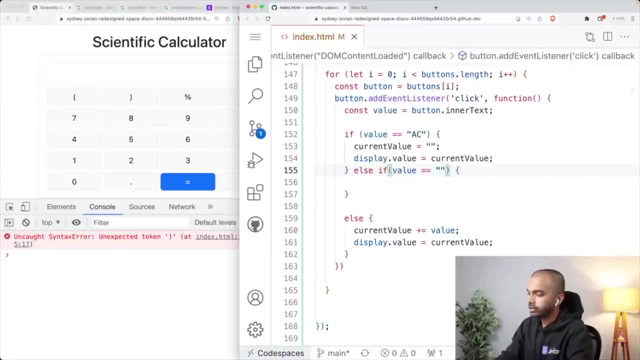 bracket over here as well And let's say: if the value is equal to the string, equal to. okay, I know this looks confusing, but we're saying the value inside, which is the inner text of the button, is equal to the string, equal to. in that case, what do we want to do? Well, let's maybe write: 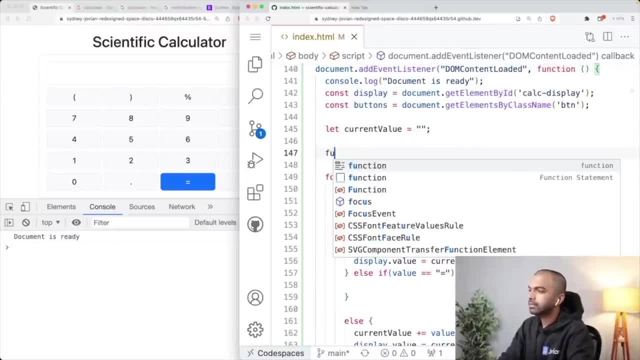 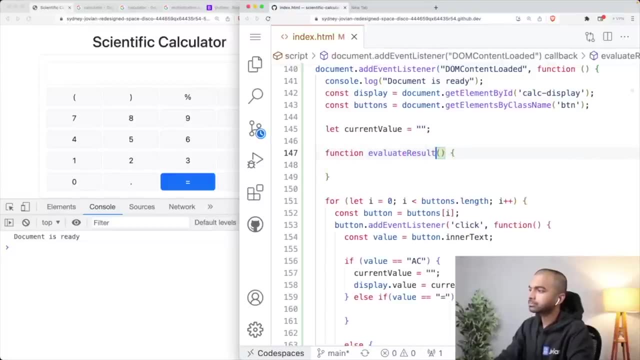 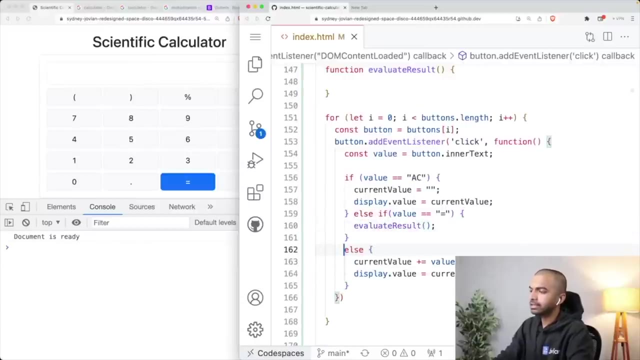 a helper function here to do this. So let's see, Let's call this function evaluate, So function evaluate, And let's call it evaluate result, And let us just call this function evaluate result. in that case, Okay, and we're going to put- and this is just to keep our code organized slightly nicely- 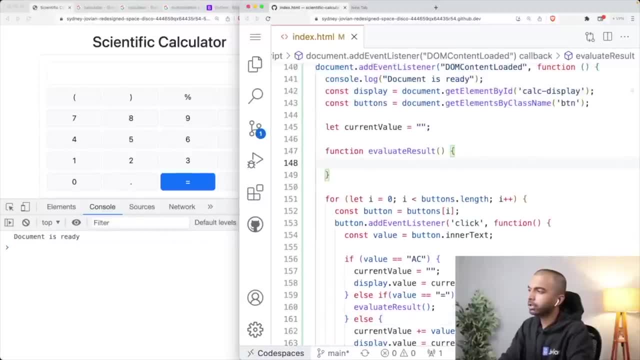 So evaluate result. So I am just gonna- here's what I'm going to do. I am going to simply say: const result equals eval. Okay, and now this is a very dangerous function. be very careful while using it. But here's what eval does you give it some. 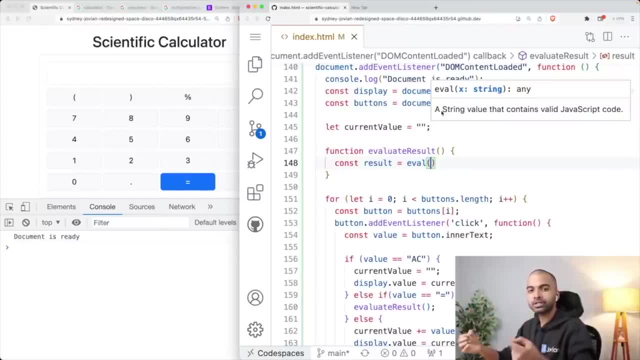 JavaScript code and it is going to execute that JavaScript code for you. Ideally, you should not be evaluating user submitted JavaScript code on your website, because they can have some code there which can fetch some data from your from somewhere on your server and then do malicious. 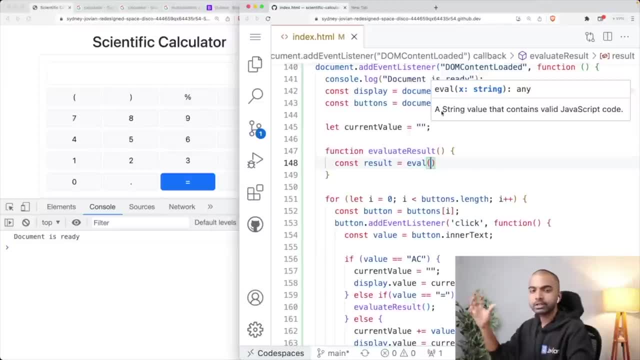 things with it If this code could be coming from some Chrome extension or something. So definitely never use eval in production applications. Rather, you might want to write an if else to kind of parse the expression and then execute it. So I'll leave that as an exercise, But for now I'm simply 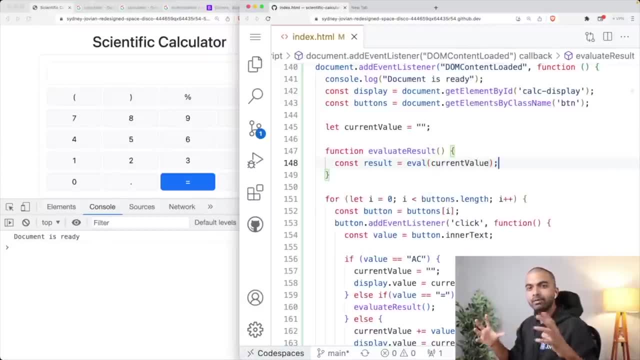 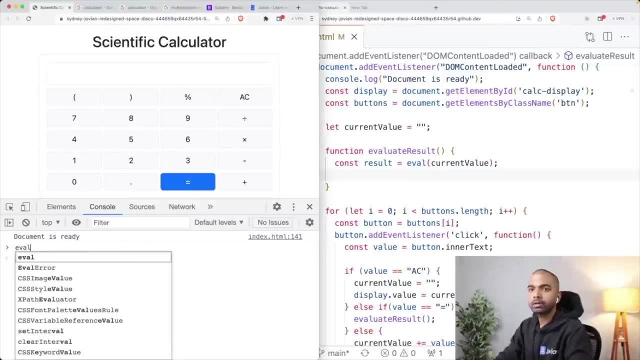 we're going to evaluate the current value. So I'm going to take the current value as an expression, as a JavaScript expression. I'm going to evaluate it And you can test this out. you can actually go into the Yeah. so let's say you, you type two plus three. you can see that that evaluates to. 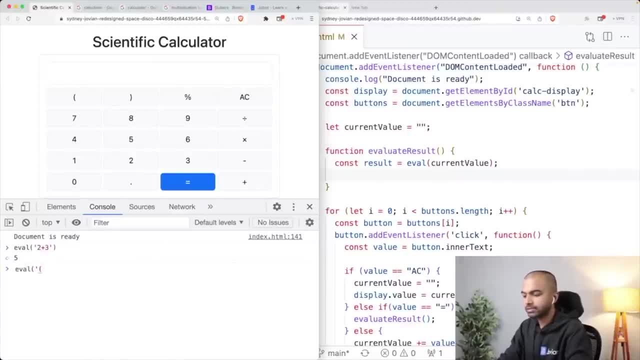 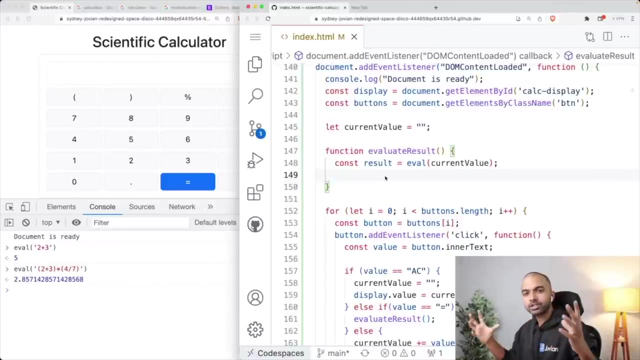 five, right. And you can also do slightly more complex things. you can say two plus three. Now, of course, in JavaScript, multiplication has this star symbol: four divided by seven, And that evaluates to 2.85, etc. Right, So eval is simply going to take an expression and execute. 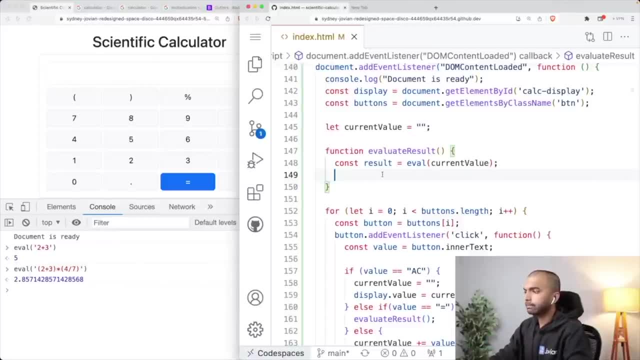 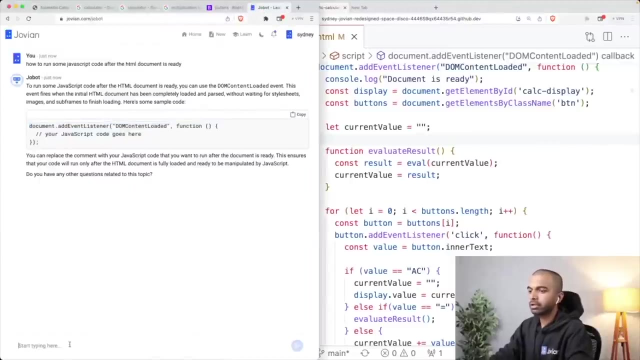 it like JavaScript code and store that result in this thing called result, Okay, And then we can say: current value equals result And maybe you can convert it to a string. So how do we convert something to a string in JavaScript? I'm just going to add: ask jobot, How do you convert something to? 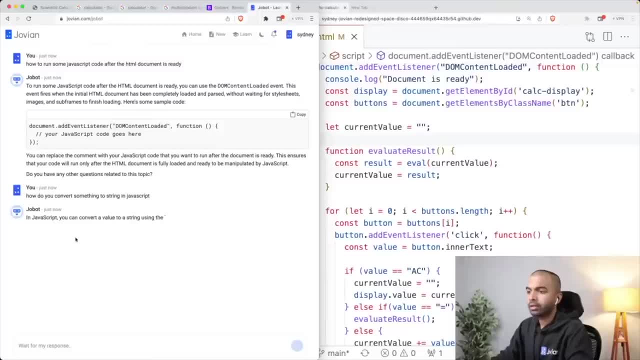 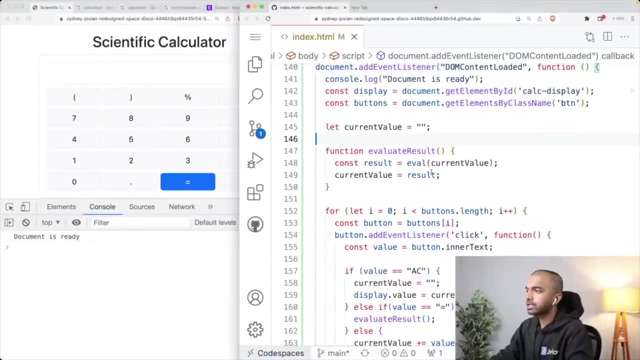 string In JavaScript And you can just say dot to string and that's going to convert it to a string. So I'm just going to use that. So I am just going to say result: dot to string. Perfect, And let me now set. 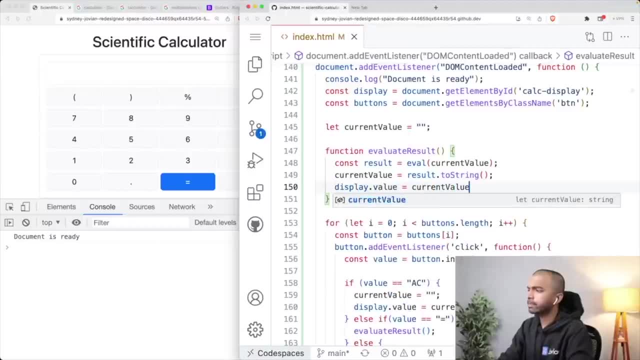 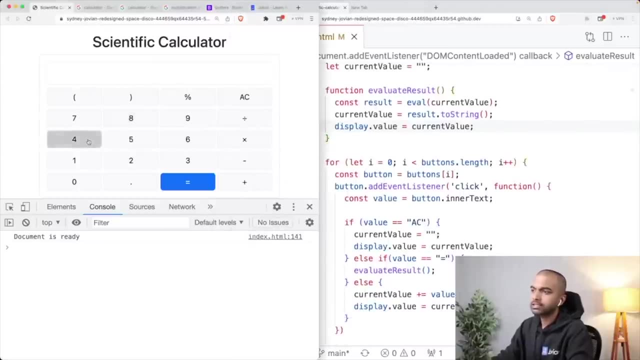 display: dot value equals current value, And I think this should be it. Let me also maybe, Yeah, let's, let's try this out first. So let's say: four plus three equals seven. Just like that we've implemented our calculator. see what? that wasn't that hard, and we are still. 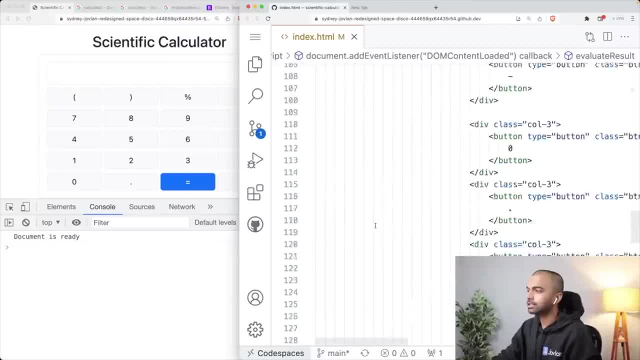 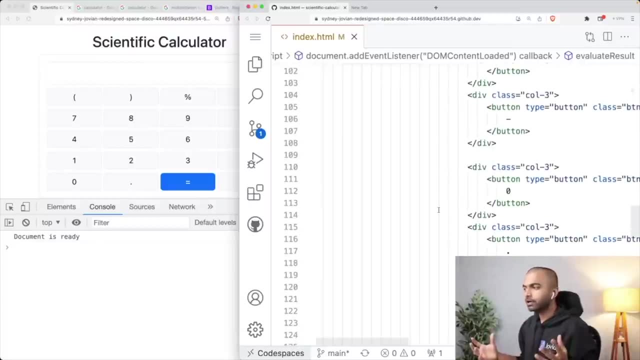 just about at 160 lines of code, But of course, most of this code is just a bunch of buttons copy pasted many, many times, And we will. when we learn frameworks, we are also going to learn about how you can reduce the amount of HTML that you write where you don't have to copy paste. 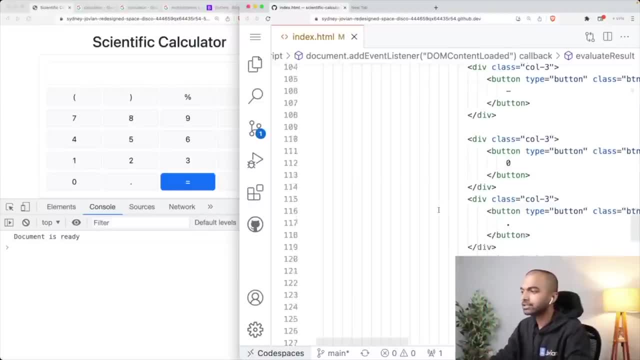 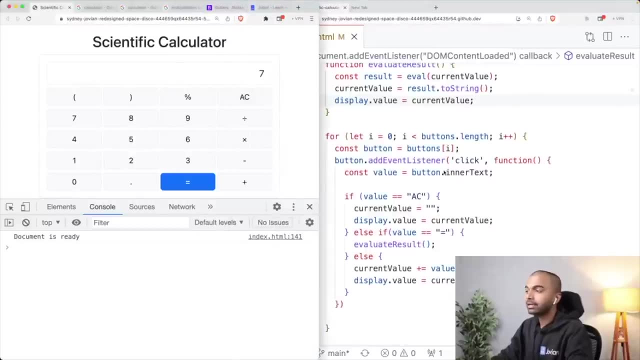 things, And if you have to change the style of all the buttons, you have to go and change them in a bunch of places. But for now, since we're keeping things simple, let's just keep it that way. But just like that, we've implemented the functionality and it works. 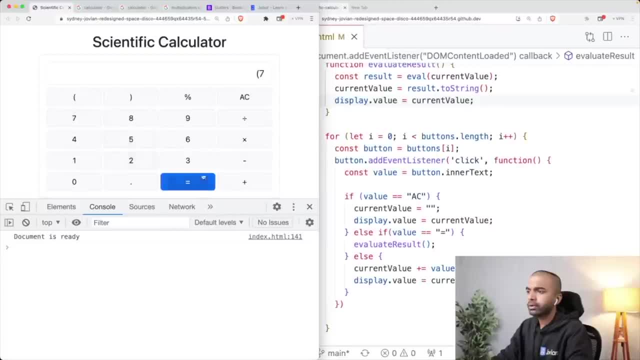 probably with something even more complex. I could say seven minus three plus, and then, in brackets, 2.1 plus six, And that entire thing works Okay. so that's good. There is one problem, though: AC works as well. Let's try eight multiplied by nine. What does that do? Okay, that fails. 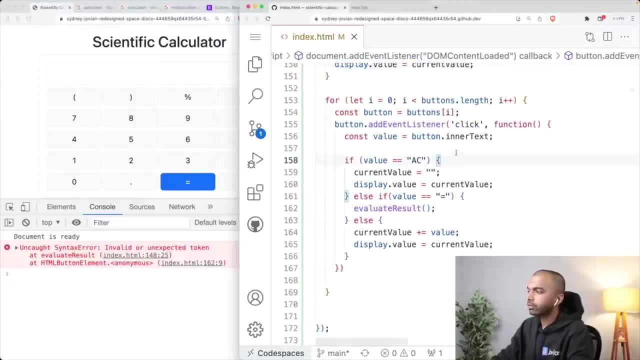 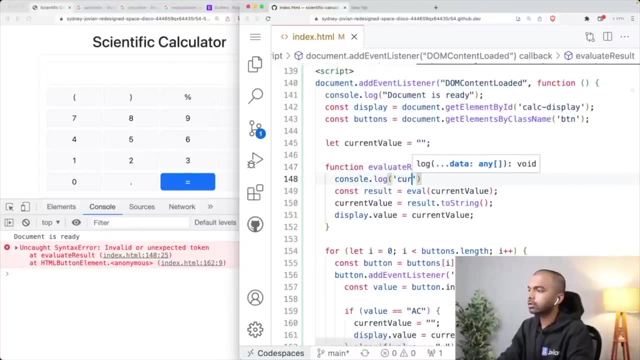 And that fails specifically because, well, inside evaluate result, let us just log the value of current value. So let's say: console dot: log current value, Current value. Okay, it's always a good idea to give labels to your logs. Let me get rid of this document. dot is. 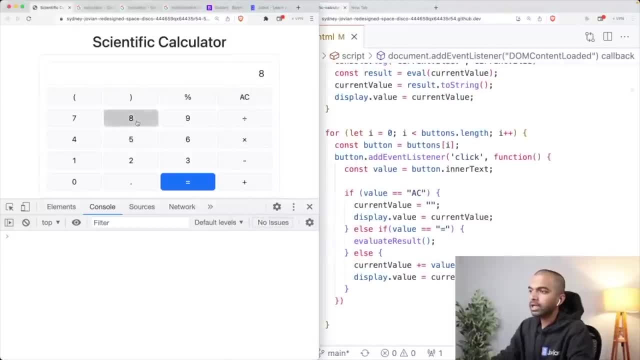 ready. I think I don't need that anymore. Okay, so when I do eight times six, you can see here that the current value is eight times six. it has this time symbol, but we don't want the time symbol. we actually want the symbol. 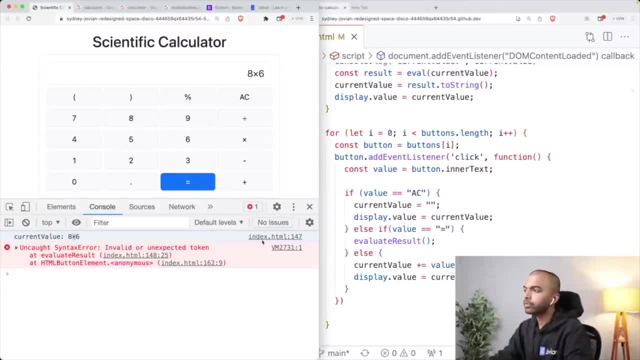 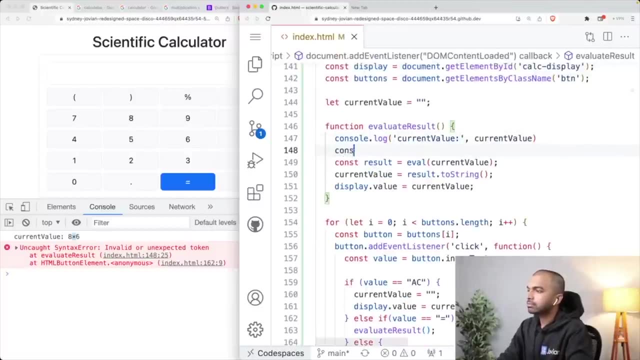 star. the star symbol is what is valid JavaScript code, So we may have to do some replacement over here, And that is where we can say const. Let's see converted val. let's just call it: converted value equals current value. So current value is a string And in the 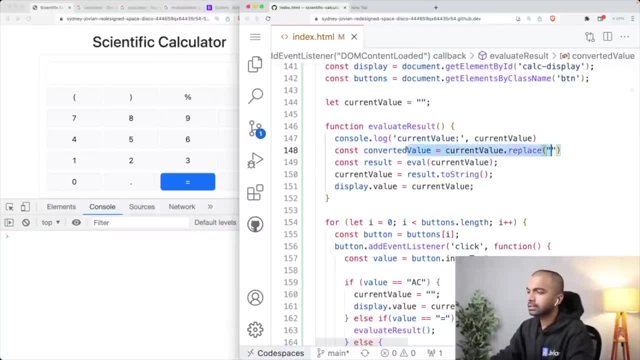 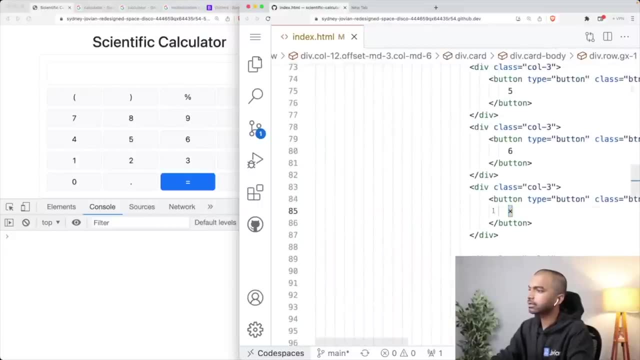 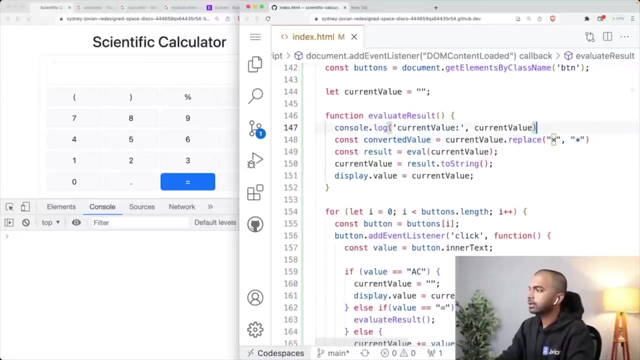 string. we simply want to replace those the this character over here, which is the times character. let's get that from our code over here. Yeah, so this is the times character. So we want to replace the times character with a star. Okay, so that's all we're doing here, And now we oops. 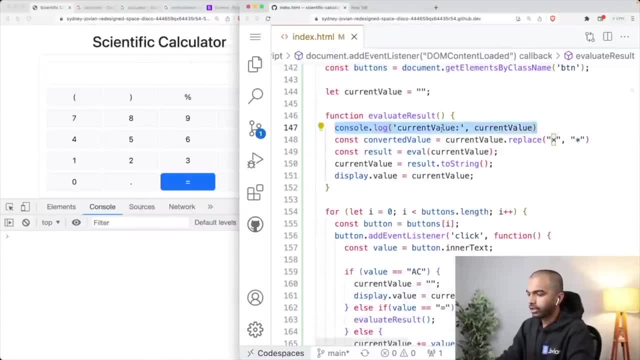 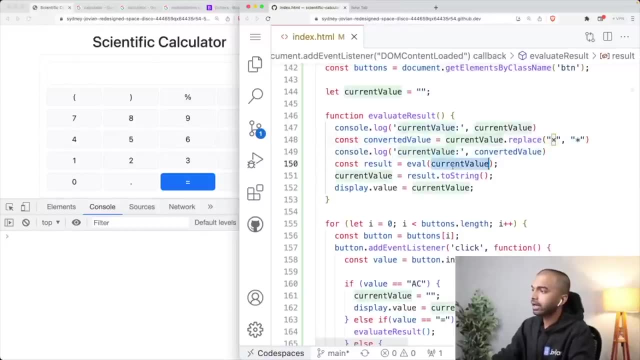 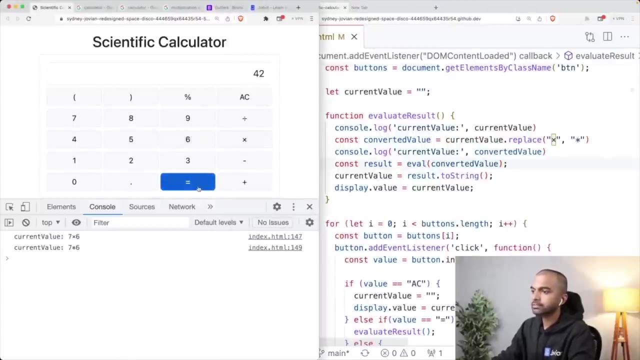 sorry about that. And now we can log the current value. And let's log the converted value as well. In the converted value we've simply replaced times with star And let's evaluate it. Let's evaluate the converted value. Okay, so let's now tie seven times six equals, And you can see here that the current volume is. 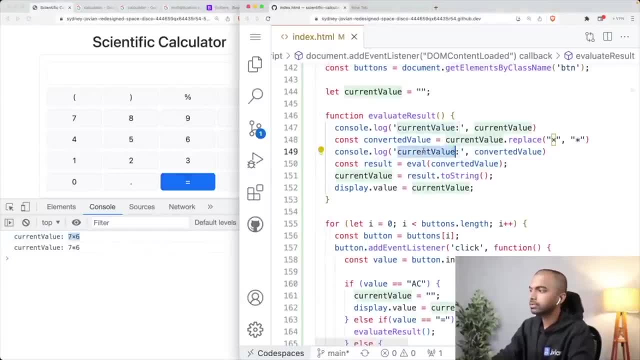 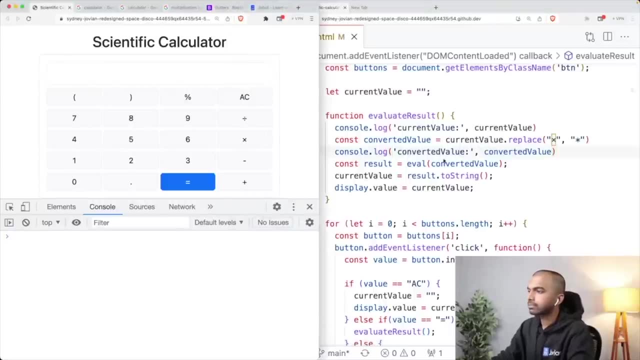 seven times six and the converted value- they should say converted value- And the converted value is- let's try that again- nine times six. So the current value is nine times six and the converted value is nine star six, which is valid JavaScript code And that ultimately ends up being converted into: 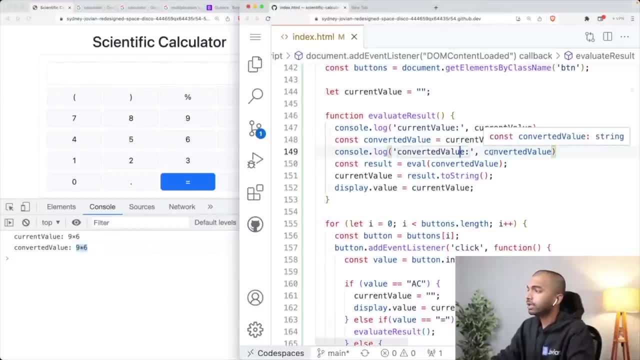 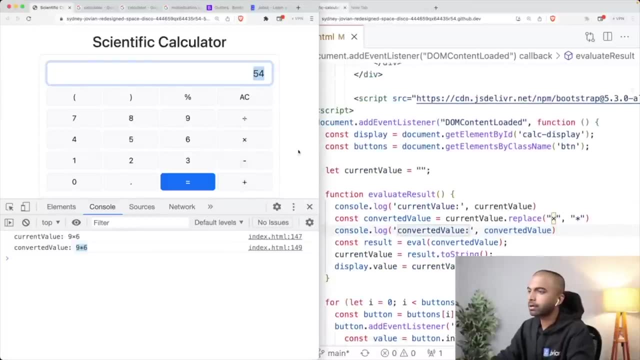 the string 54. Okay, so that's great, We have fixed that. Maybe there's. we also want to fix the division symbol, So let's go ahead and fix that as well. We don't need to fix minus and plus, they're probably fine. We probably need to do something about the percentage as well. We're 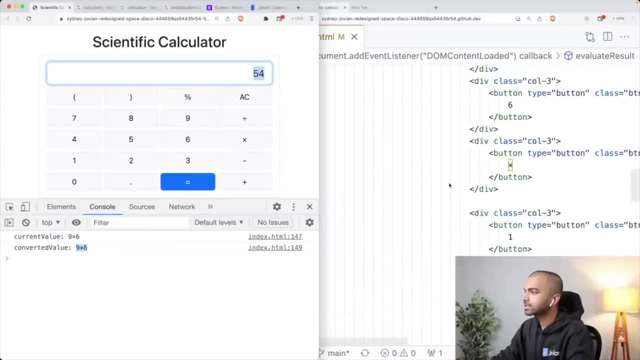 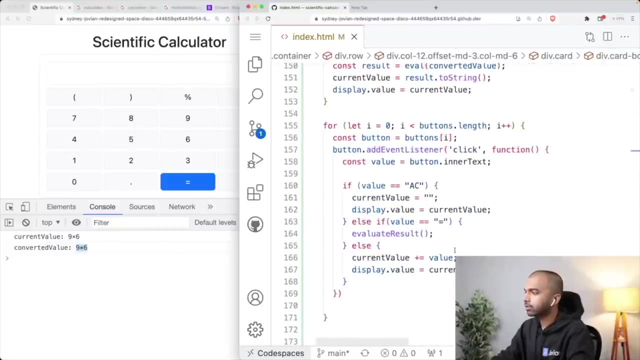 going to see what to do about that, But let us fix the division symbol. Let's go ahead and fix that. Let's fix the division symbol as well. Let's grab the division symbol over here And let us come in here And let us just go in and say: 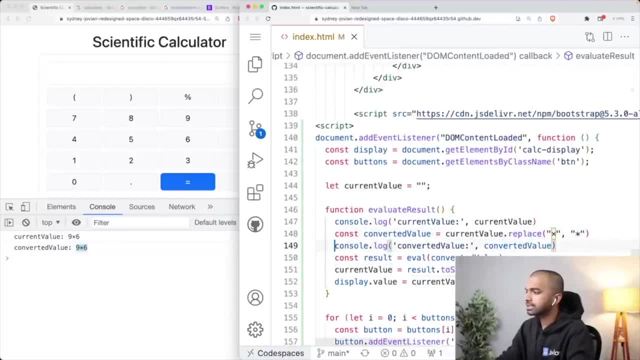 yeah, replace right. So I'm just gonna come in and say, let's, let's add some space here, just so that things are a little easier to see. And, by the way, in JavaScript you can actually put statements on the next line, just for better readability. So I'm simply replacing the. 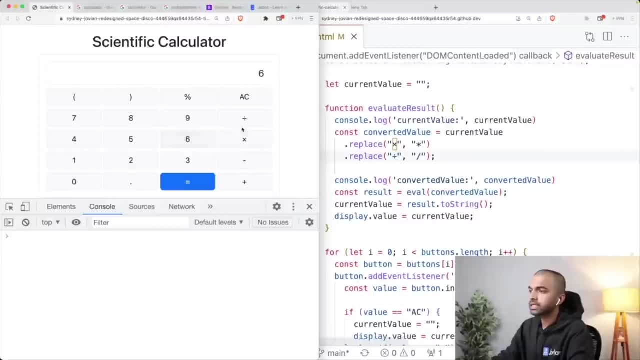 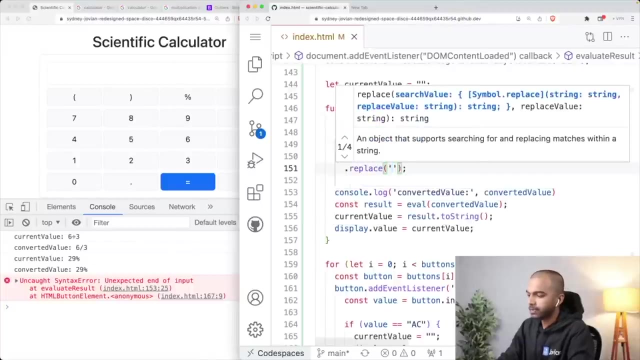 division symbol by slash. Hopefully now, six divided by three should work. That's two. Let's write: percentage of 929% equals okay. that doesn't work again. So we want to convert percentage as well. A quick replacement for percentage would be to simply multiply by 0.01.. So I could just say: 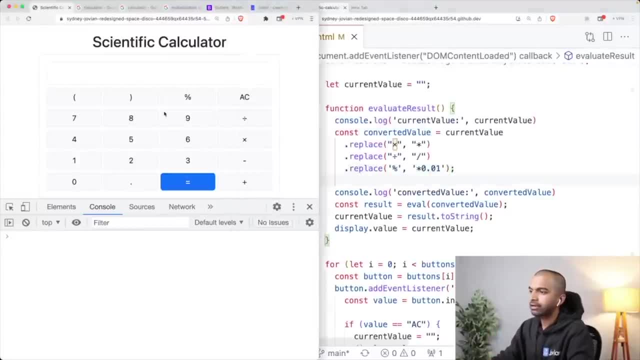 multiply it by 0.01.. And let's see now. So let's see: AC 9% equals 0.09.. Okay, that's working As well. I think that's it. That is our basic calculator. We've not added the scientific. 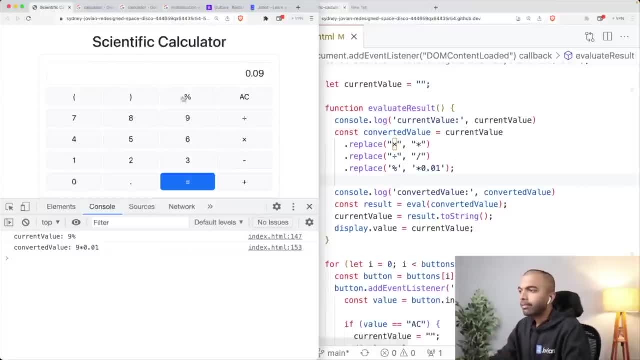 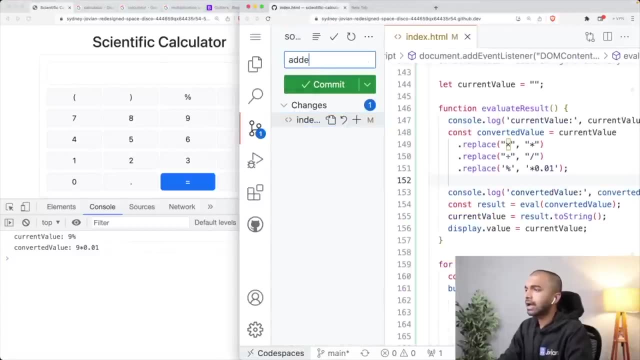 functions yet We will see how to add them in just a bit. But that's looking pretty good And things are looking good so far. So I'm just going to commit this. So I'm gonna say added basic functionality And let me just commit that And let me send that back to the 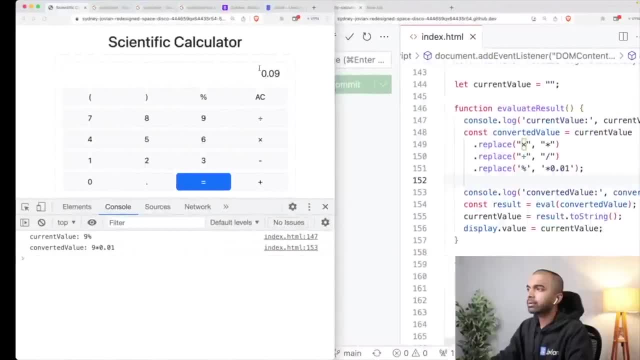 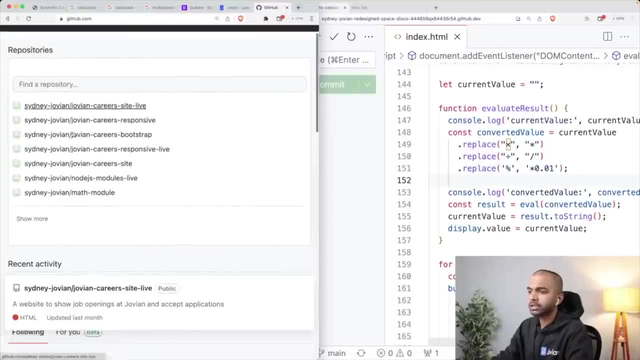 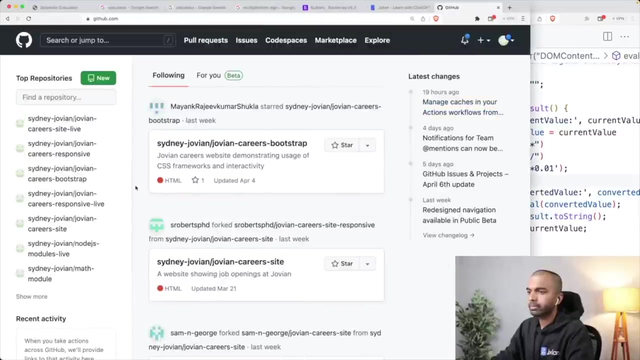 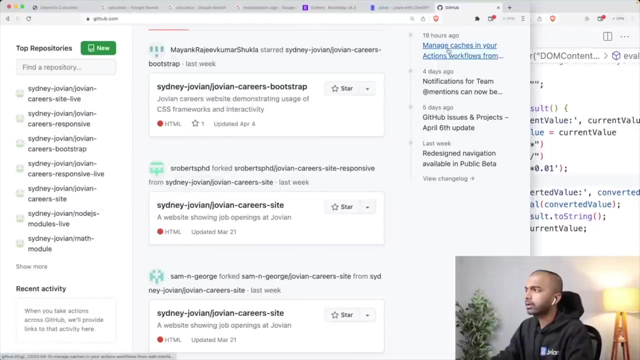 GitHub repository. Okay, Now I can check back the GitHub repository. So I can check back the GitHub repository over here. Let's see githubcom and I should have my repository here. Where is it? Well, I'm just going to go into my profile and in my profile I'm going to look. 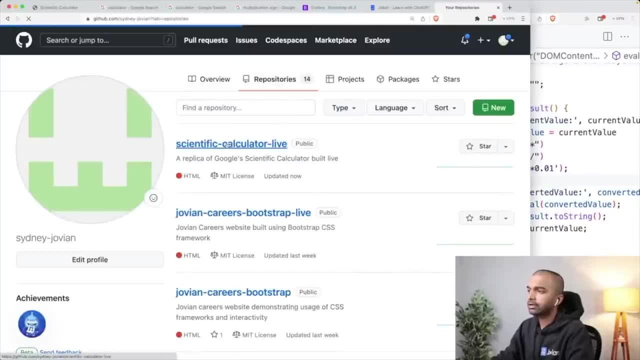 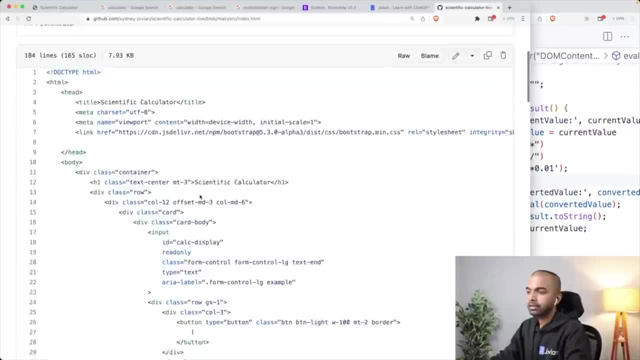 for repositories. And here we have scientific calculator life, And you can see scientific calculator life has all the code and everything is still inside indexhtml. One quick thing I'm going to show you right after this is how to separate out the script into a different. 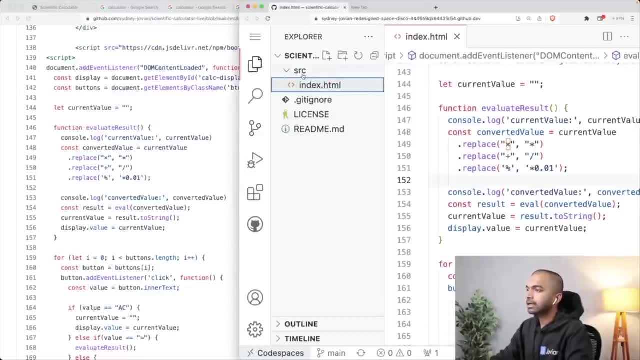 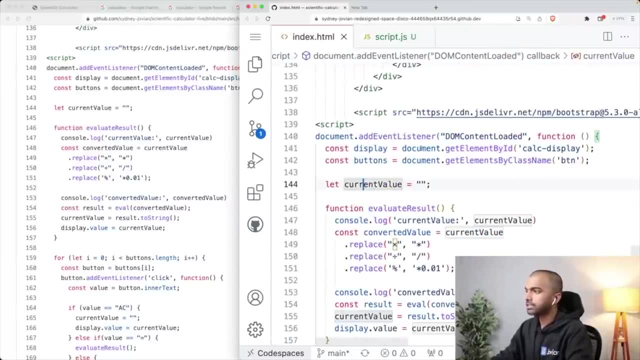 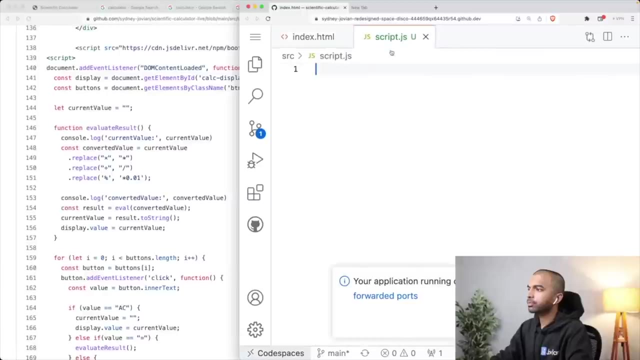 file. So let's do that as well. Let me come back in here. Let's create a file- scriptjs- and let's grab all the code from indexhtml into scriptjs, Okay, And let's put that in here so that we can. 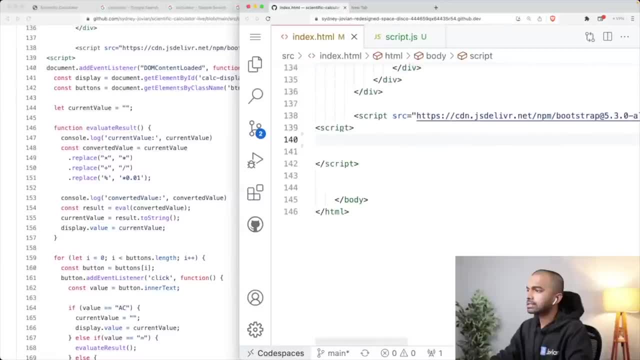 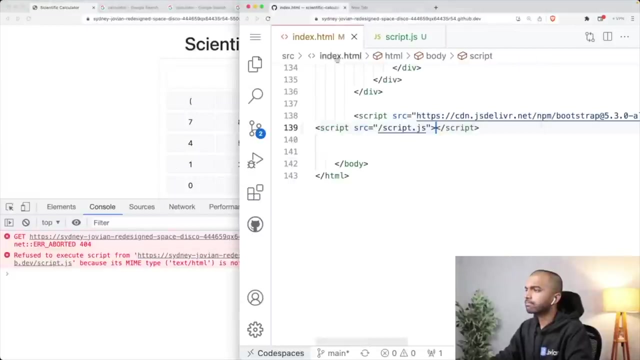 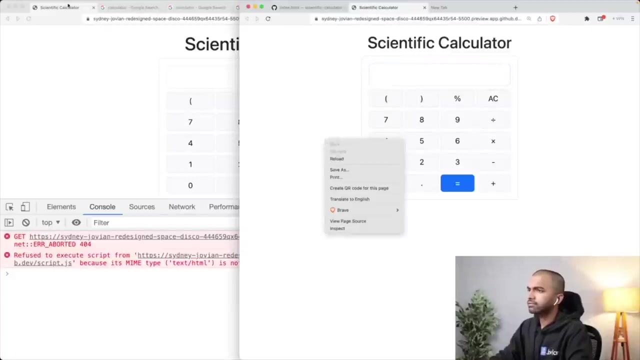 worry about it separately, And let us now just give this SRC equals scriptjs. Okay, And it should still work exactly the same way. Hmm, Let me just restart the live server And let's see. Okay, Let's try going live again. Yeah, There it is, And let's see if the let's grab this and 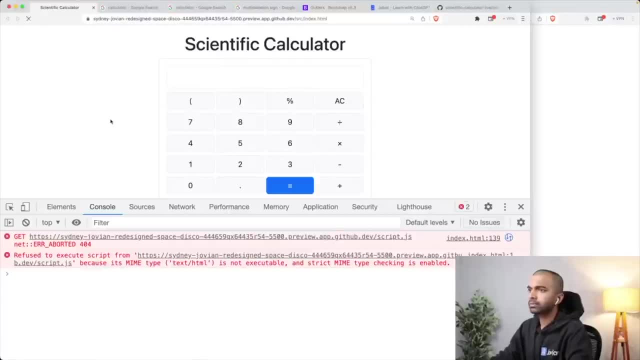 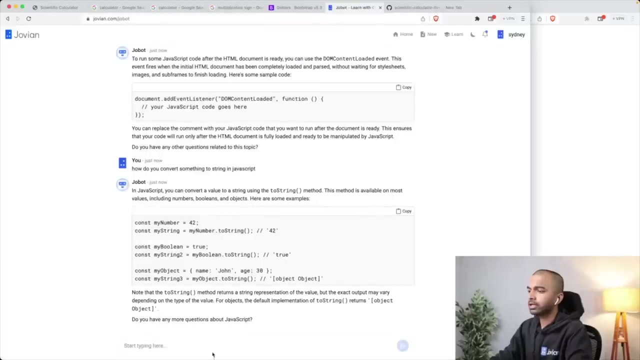 put it in here. Okay, Okay, Okay, Okay, Okay, Okay, Okay. I believe it's working Well. it says: refused to execute script fromWHAT Let's. we should be able to fix that, So let's just go into Joet slot and let's search. I got this error while including: 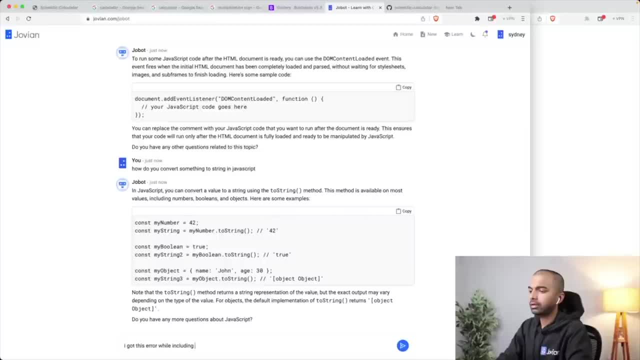 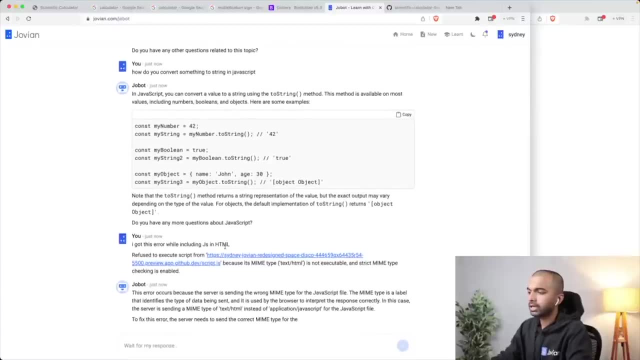 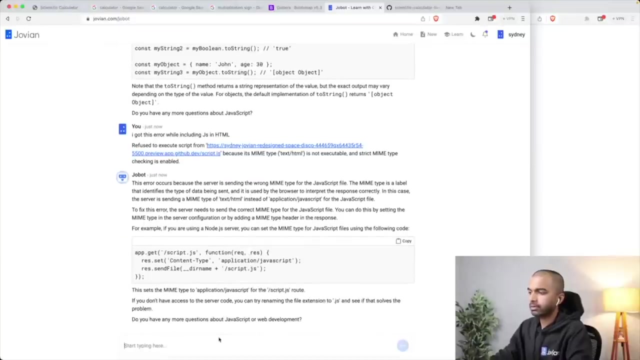 This is fun. This is actually working And it 안녕. Okay, And so it's working. I'm not going to我在 amount yet, Okay. Okay, looks like there's some kind of a. Yeah, I'm just gonna say I don't have access. 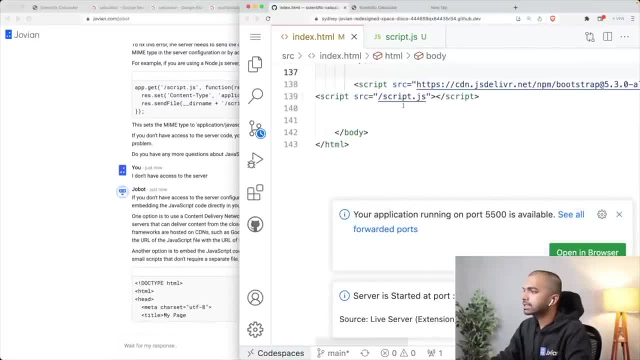 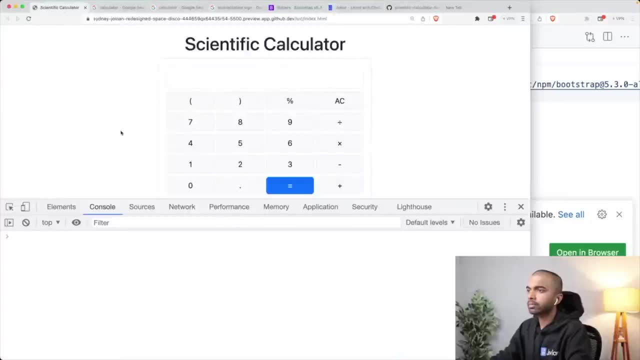 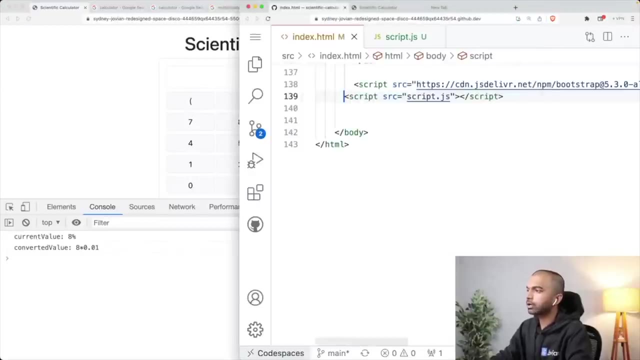 All right. well, looks like there's probably nothing I can do about this at the moment, So I'm just gonna have to maybe bring back my JavaScript code. Well, no, it's gone. Okay, Yeah, that did it. I think I just had to put src scriptjs instead of slash scriptjs. 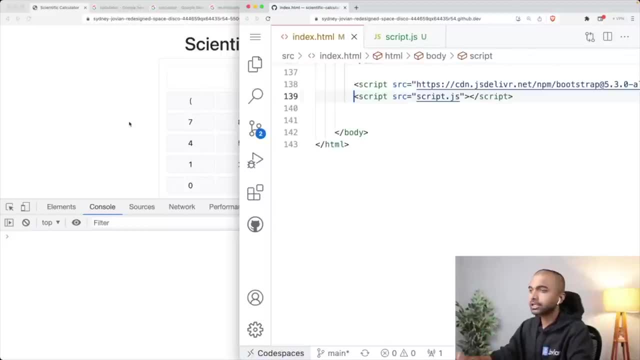 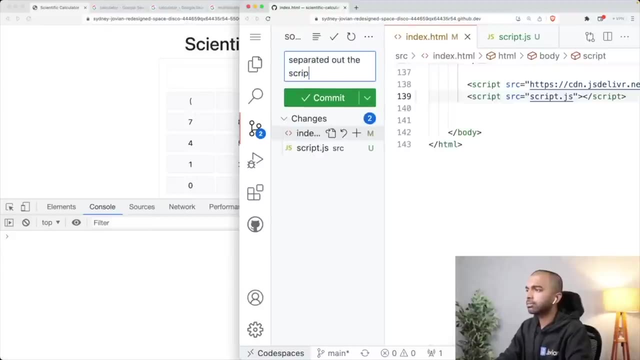 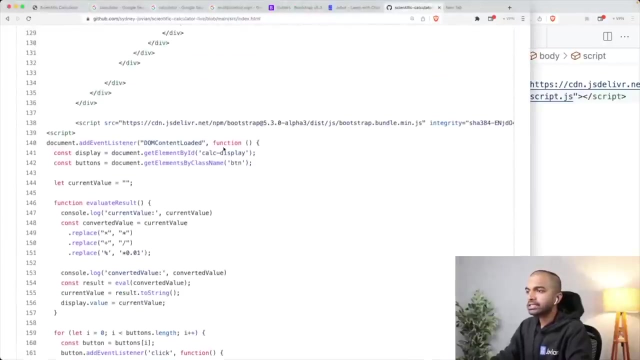 And that worked. Yeah, sometimes you run into these errors and you just search online and you should be able to figure them out And let us just commit this. So let's say, separated out the script file And let's push it back. And now the next thing I want to show you. 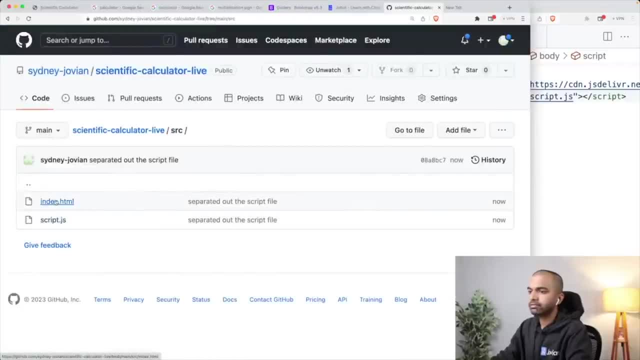 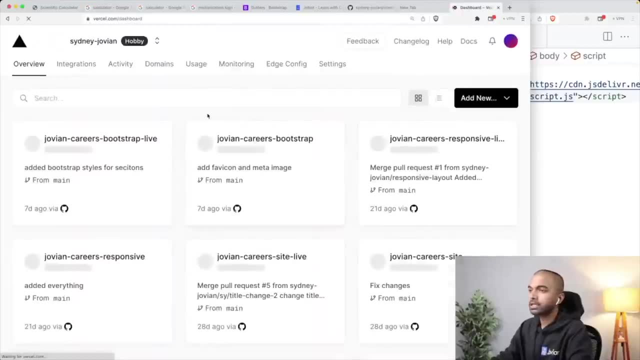 now that this is loaded up, let's just: yeah, you can see there's an indexhtml scriptjs. I want to show you how to deploy this So you can go to Wurselcom and create an account, And Wursel is a platform for very easily deploying. 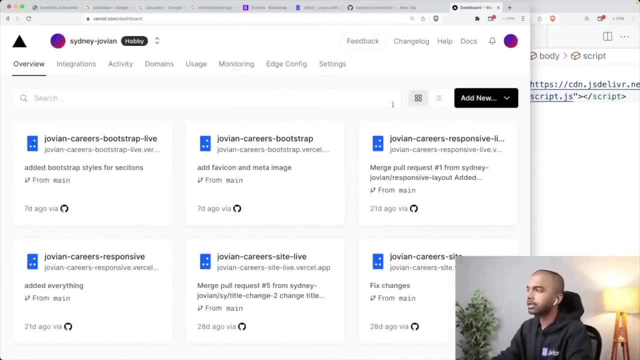 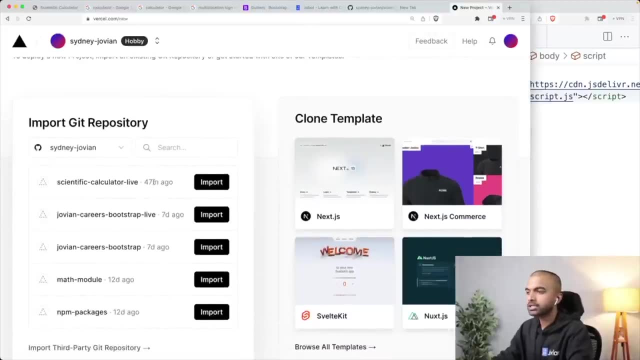 JavaScript related or node js projects in any web web related project And I'm going to say add new project And you can connect your GitHub account here and can get access to your private repositories, public repositories, etc. And you can see here that it can see in my 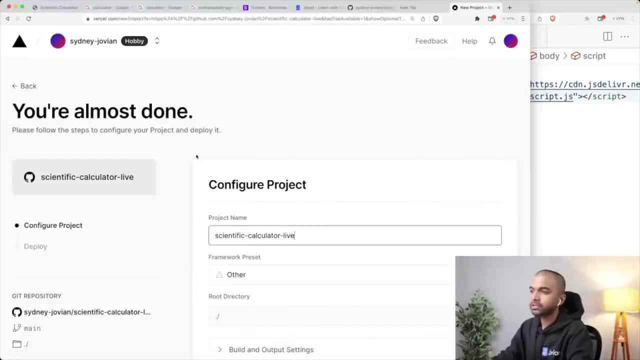 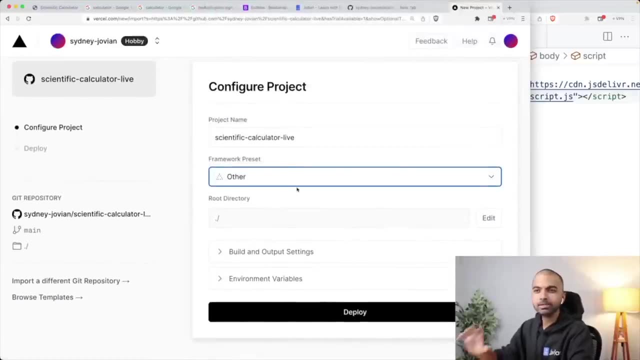 account that there is this scientific calculator live, So I'm importing this project over here And here on Wurselcom I can select some frameworks. I'm not using a framework right now. there's a CSS framework, but this is talking about more of a backend framework that I'm using. 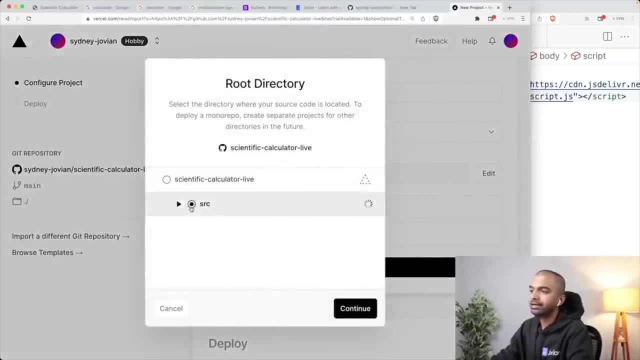 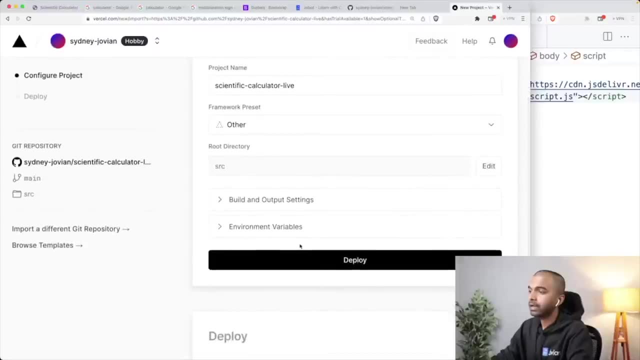 I'm not using any of these, But I do need to tell it which directory contains my indexhtml file, And that happens to be SRC. So I'm going to select the SRC directory as the live directory And then I can just click Deploy. Okay, it's as simple as that. you go to Wurselcom. 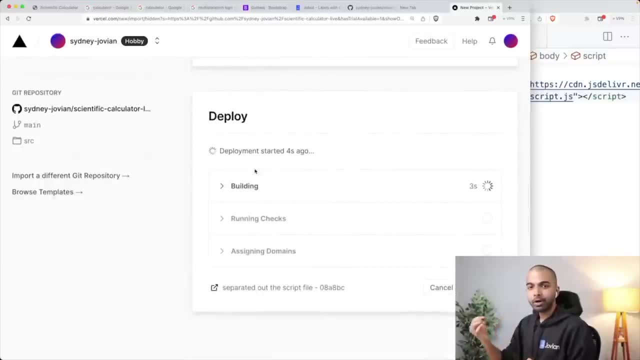 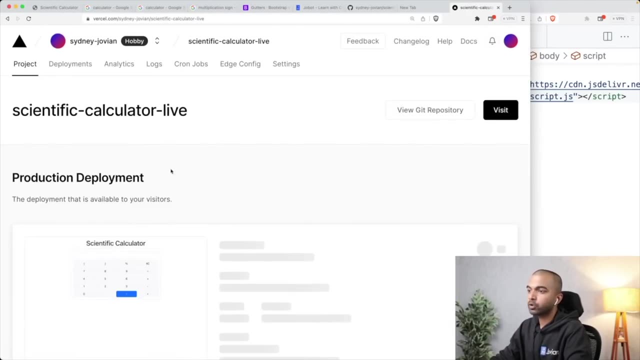 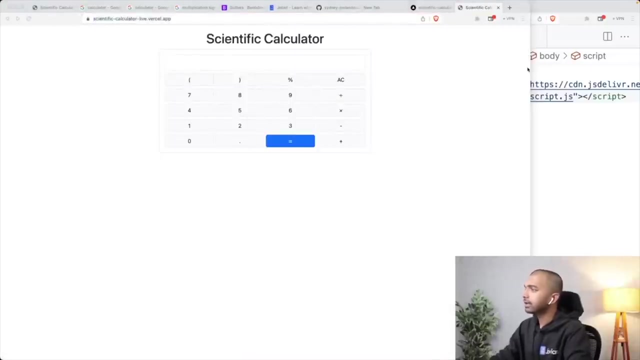 sign in, connect your GitHub with it and then click Deploy- create a new project- and select the root root directory. And now you can actually go ahead and you get this nice URL scientific calculator livewurselapp, And I'm just going to drop that in the chat And you can try it out. 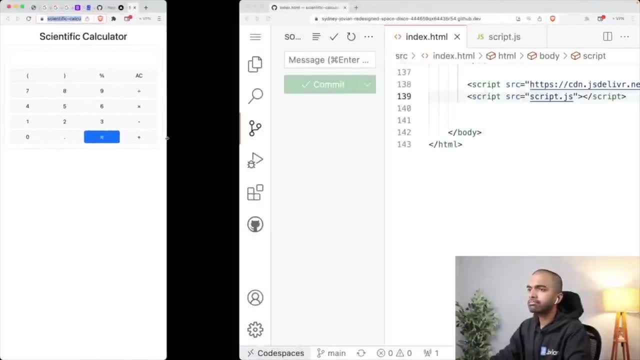 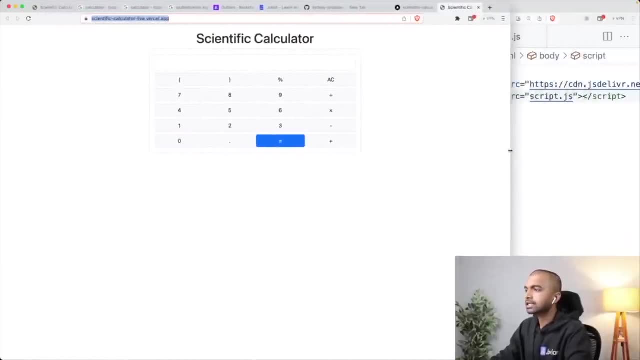 you can try it out on your own And you can see whether it's mobile friendly or not. Yep, it looks fairly mobile friendly to me, Yep, And we'll have to figure out how to make it exactly like the Google scientific calculator, But for now I am pretty happy with how this is. 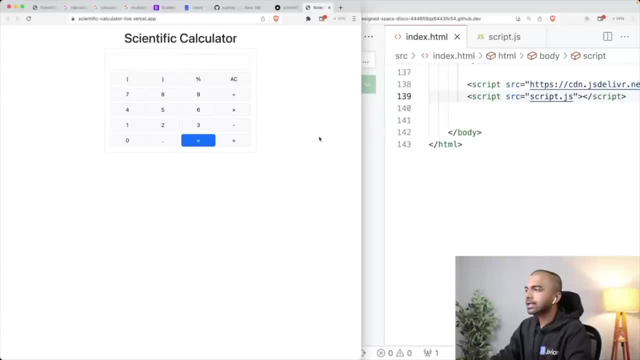 looking Okay, great. So now let's continue On. now that we've done this deployment as well, let us continue and add maybe some of the scientific features. we may not get to everything. we are kind of running out of time here as well. 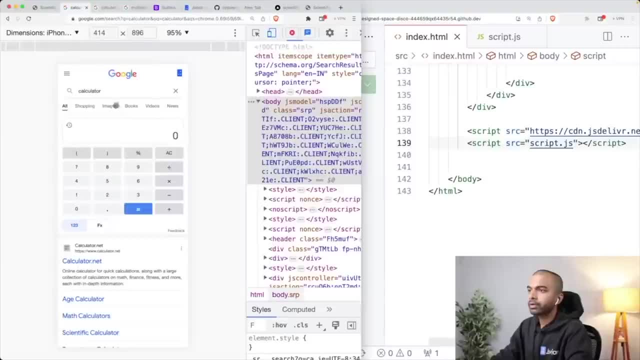 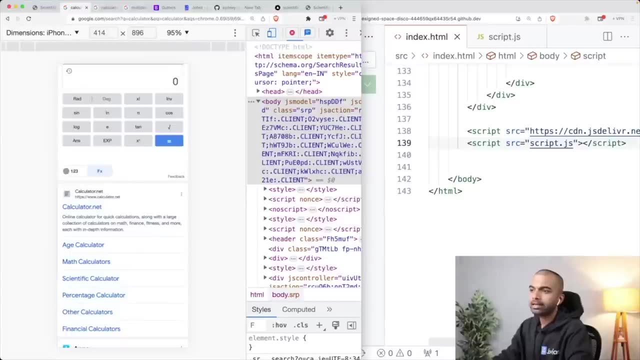 But let's see, let's add maybe a couple of rows. Alright, so now there is this selector here: 123 and FX. I'm just going to add it below. I'm just going to keep keep things simple for now, But I encourage you to try it out. And I'm going to add this row sine ln, pi and cos, because these 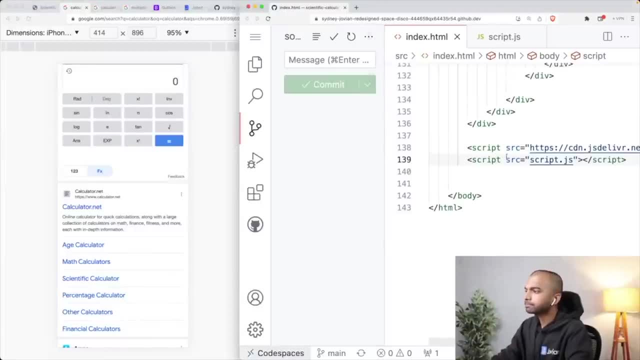 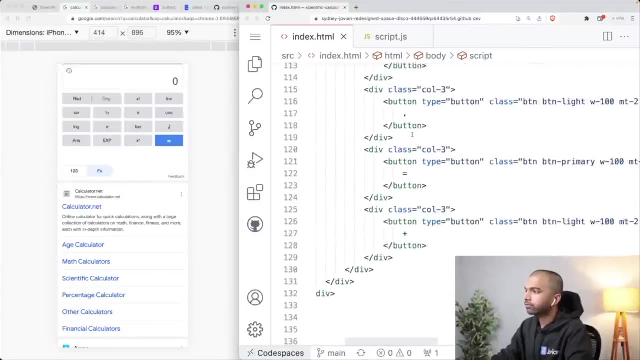 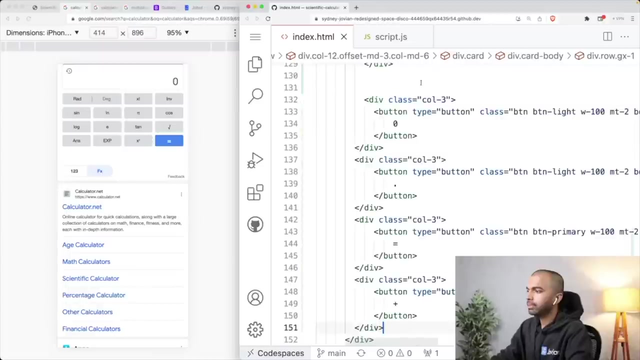 seem like an interesting set of things to add. So let's see, Come back over here And let us say, let's add another row of values. So let me grab the last four buttons And let me create a copy And let me paste that in here. So one is called sine. 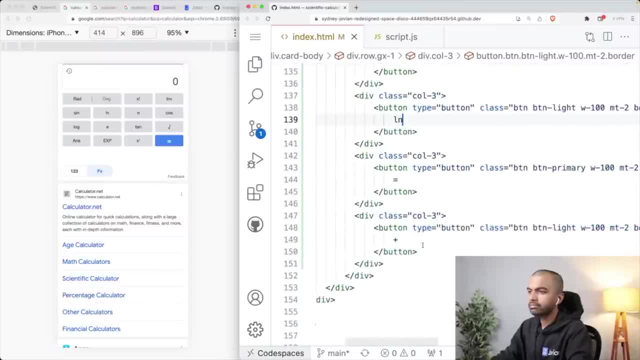 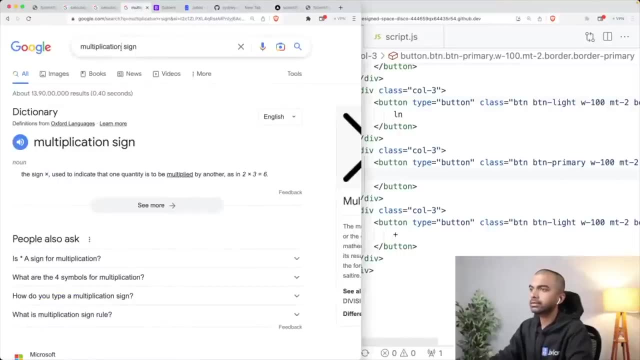 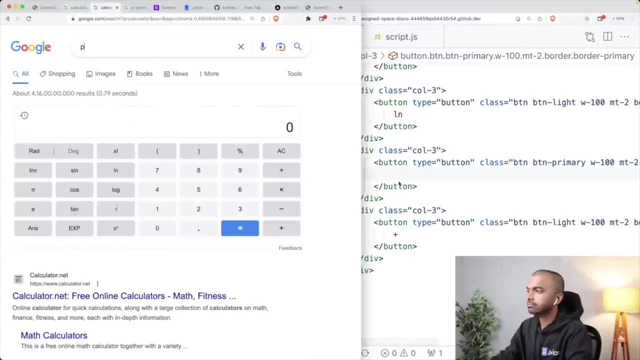 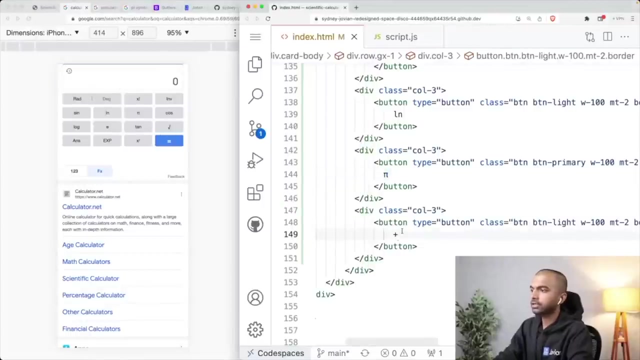 then one is called ln, which is logarithm, and the natural logarithm probably, and one's called pi. let me just get the pi symbol. Let's get it here. Archer is just that character, And let me get in. What's that last symbol over there, cos? so let's get course in here as well. 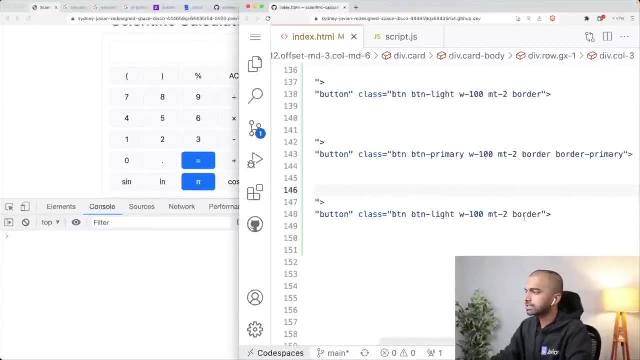 Okay, so let's see if we are able to make that work. Of course, with this doesn't need to be a primary button anymore. This can be our normal light button. Alright, And yeah, there we have sine ln pi cos and�� 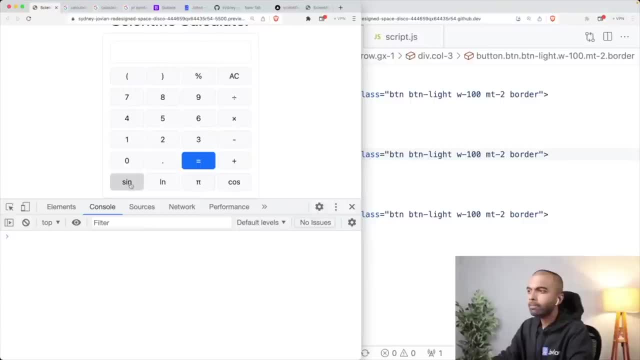 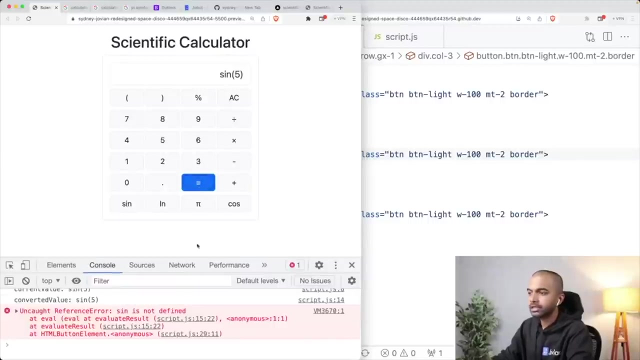 And let's try to just implement sign for now. Okay, what if we do sign and then maybe open brackets? of course, like it has to be proper, it has to be a proper expression for it to get evaluated And I click equal. okay runs into an error. So it says reference error. sign is not. 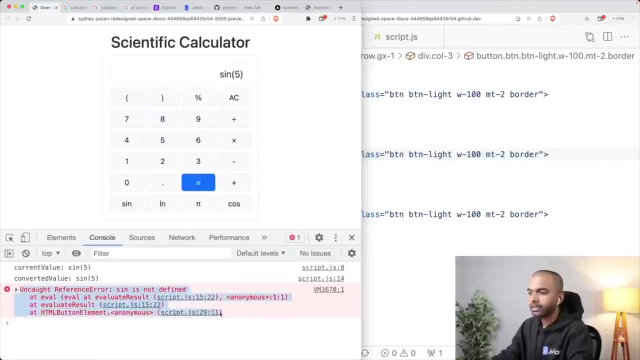 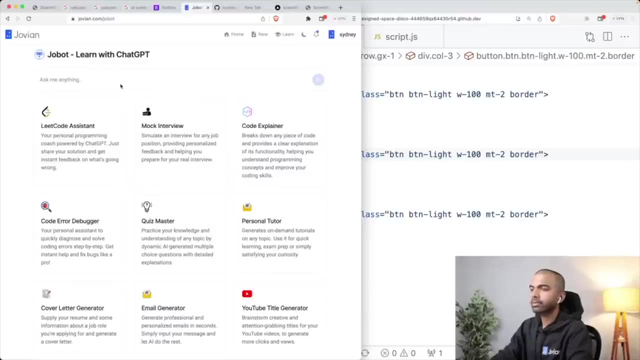 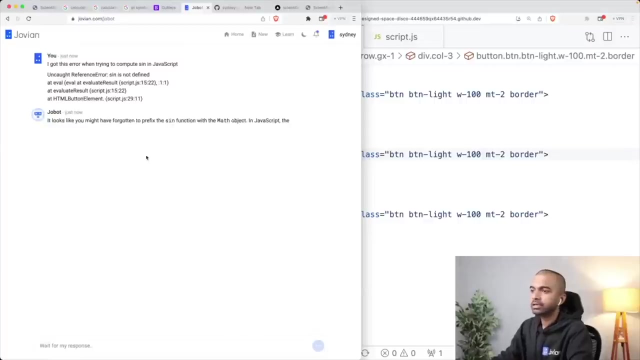 defined. Okay, And I'm literally just going to copy this error And I'm going to come back to your board and said: See, let's just reset this. I got this error when trying to compute sign in JavaScript. And what does it say? it looks like you may have forgotten to prefix the sign. 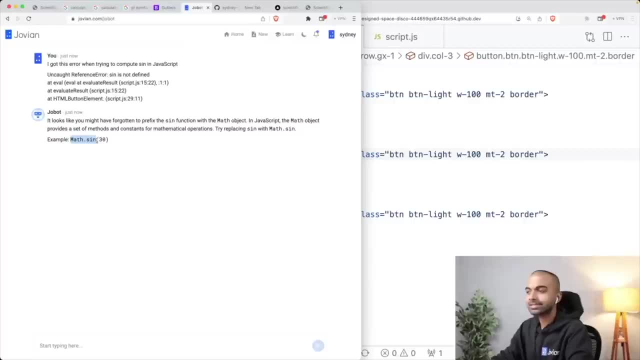 function with the math object And this is how you should be using it. Nice, So I'm just going to go ahead and use that. I'm going to go into my script dot j s and into my script dot j s. I'm just 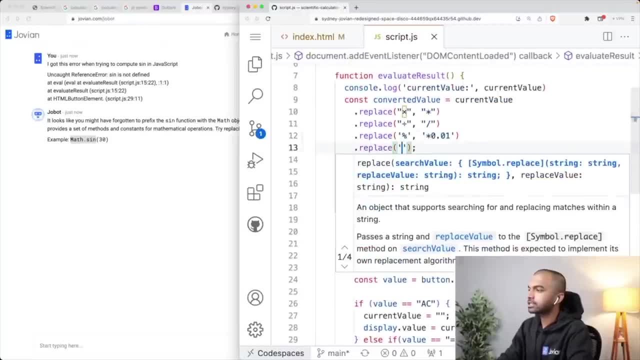 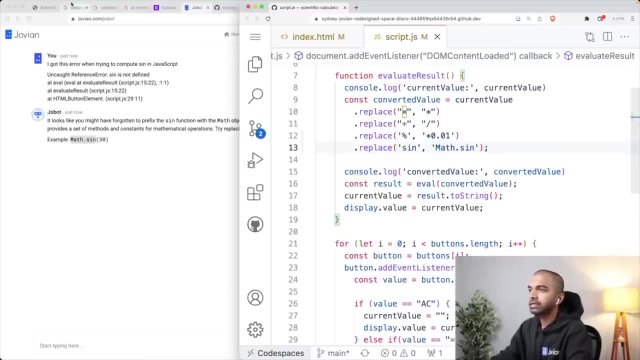 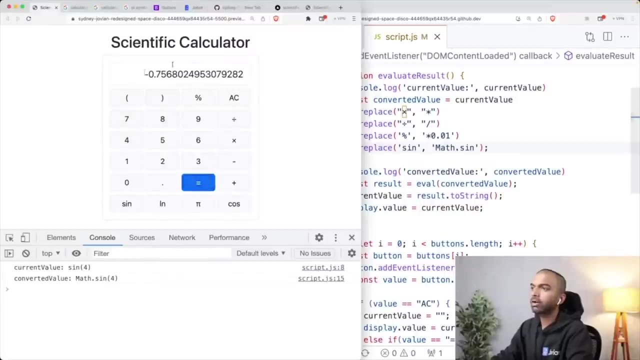 going to add that replace And for sign. I am just going to replace that with math dot sign And hopefully that should fix it. Let's go back in here and let us check. So sign for equals. Okay, looks good, It's probably in radians, not in degrees. That's fine, I'm not too concerned about. 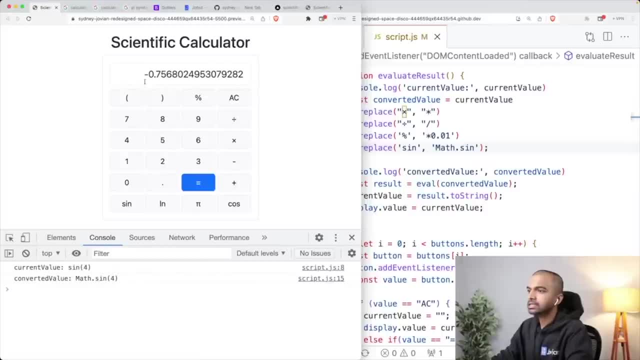 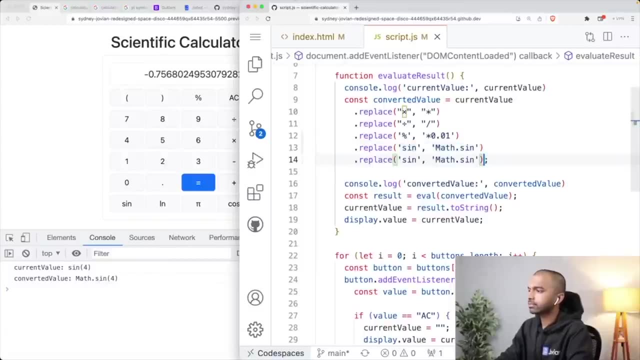 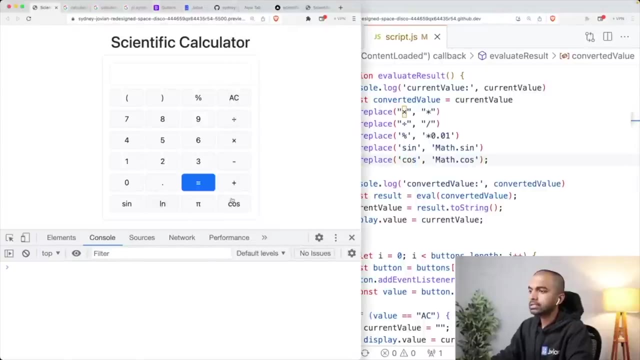 the specific details right now. So sign is implemented here minus 0.75.. Maybe we should fix costs the same way As well. Let's see cos that is simply math dot cos for cos. Okay. so let's try cos. eight times sine nine equals. 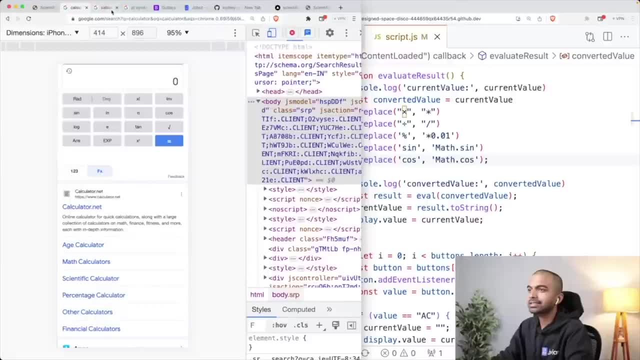 Okay, Yeah, seems fine, I could. I could just test that in this calculator as well. This calculator actually allows typing too, in case you want to try that. And it also inserts button. it also inserts a bracket and all that, So that's fine. Okay, so let's try that. And it also inserts a. 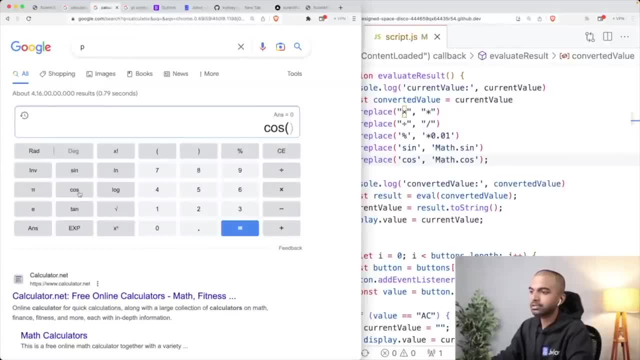 bracket and all that. So that's fine. Okay, so, let's try that. Okay, so, let's try that. And it also inserts a bracket and all that. But cos eight times sine nine. that's what we did, So cos eight? 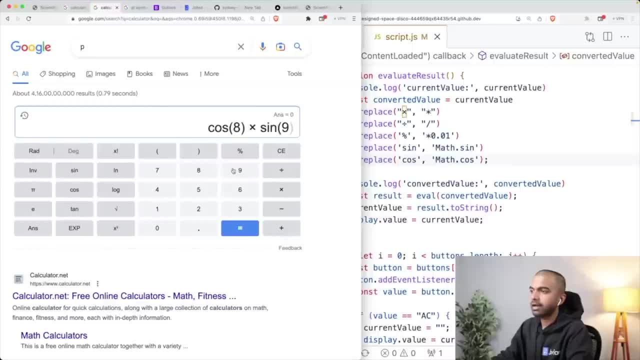 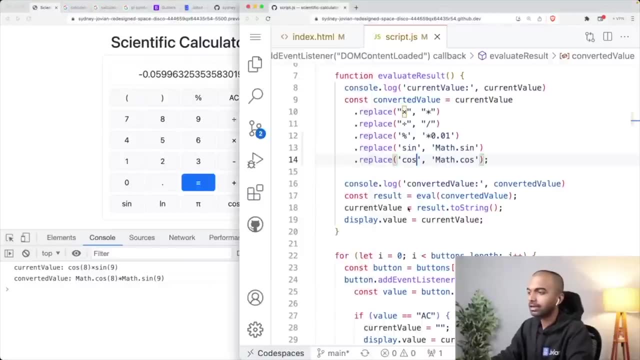 times sine nine. Yeah, that's about the same: 0.559, 0.559, 599, 0599.. Okay, that's good, Let's deal with ln over here. So, okay, I think one thing we should do is somehow find a way where. 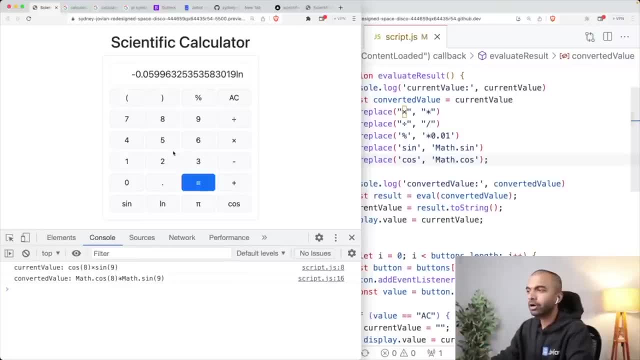 if the result has already been computed, then we should not pressing a button, should not add to that. But again, advanced behavior. I'm going to leave that for now. But ln eight, let's see if that works. No, So let's try math dot ln. I'm just going to try this out and see what happens. 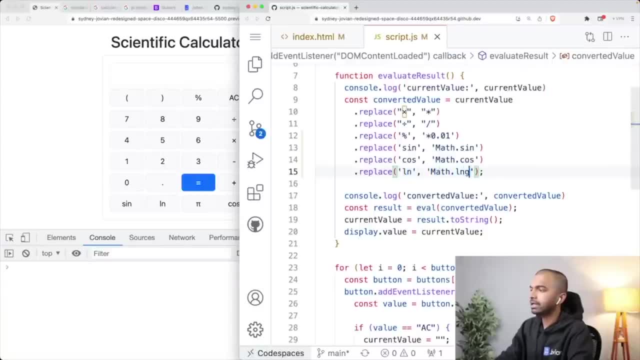 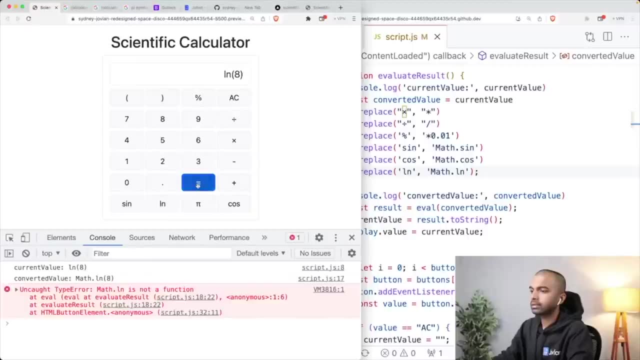 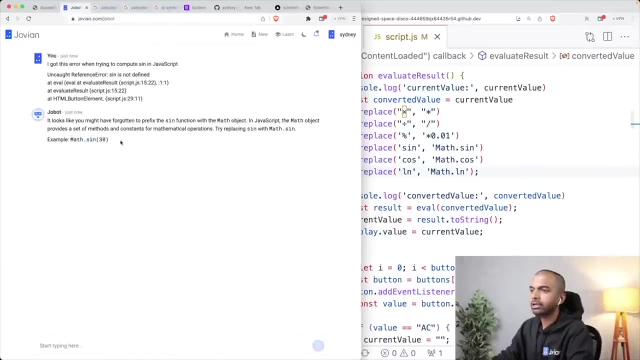 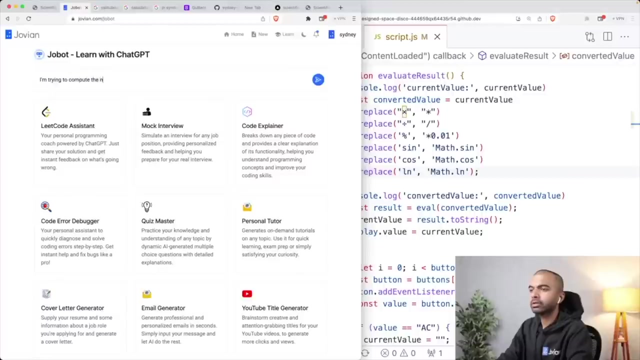 ln math dot ln. Okay, so ln eight Math dot ln is not a function. So let's see, I'm going to come back here to job. I'm going to ask it once again. I'm trying to compute the natural logarithm. 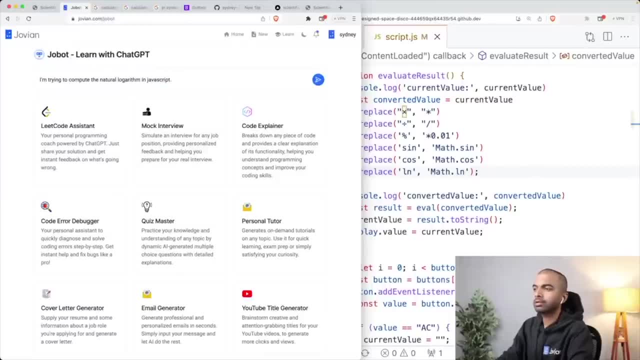 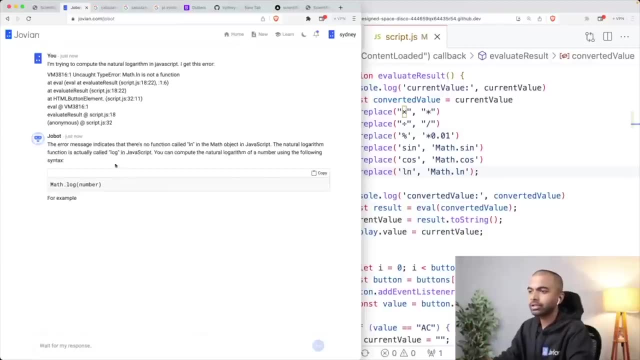 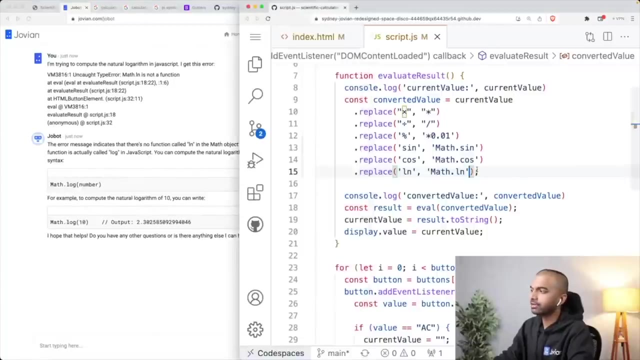 in JavaScript. I get this error. Okay, joviancom slash job. I just go in here and drop it in. Okay, it's math dot log, I believe. So for the mathematical, for the natural logarithm, you just said math dot log. So I'm going to change that to the math dot log And I'm going to say: 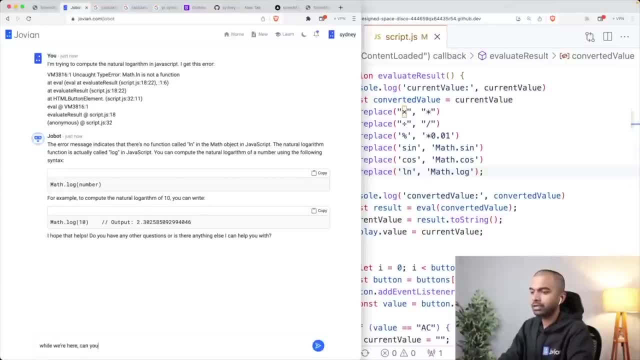 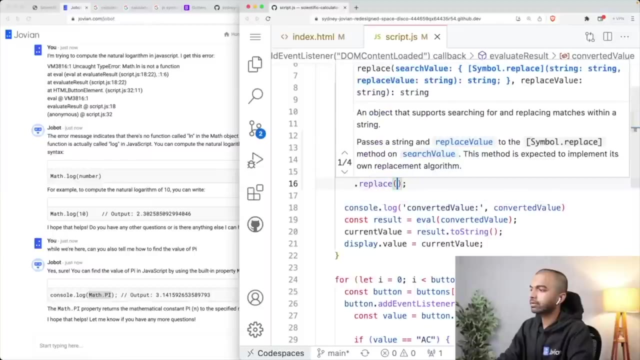 while we're here, can you also tell me how to find the value of pi? Yeah, it's just math dot pi, So I'm going to fix that as well. So let's go in here and let's replace the pi symbol. I'm going to get the pi character. the pi symbol is right over here. 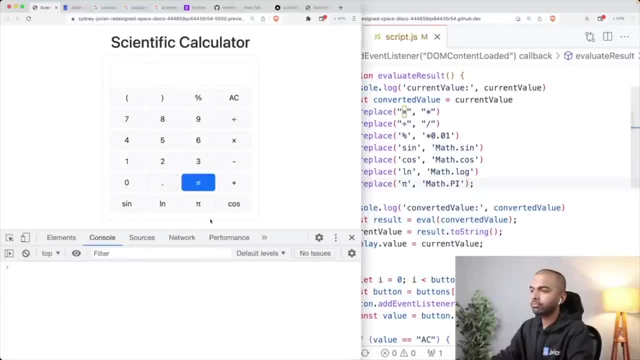 And there you go. We have fixed that as well. So now we type pi, you press equals, that's 3.14.. And whatever pi means, okay, And we can, for example, try to compute the the pi r square of a circle. Okay, that reminds me we can probably add things like square to. 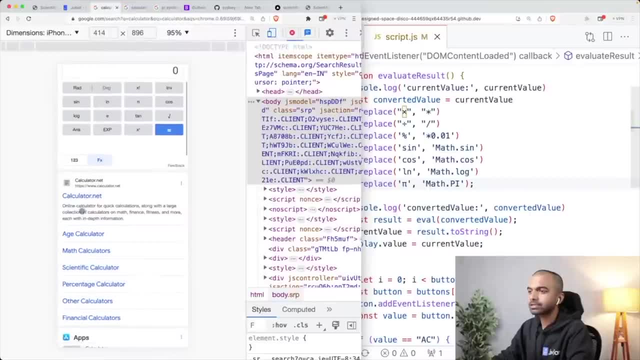 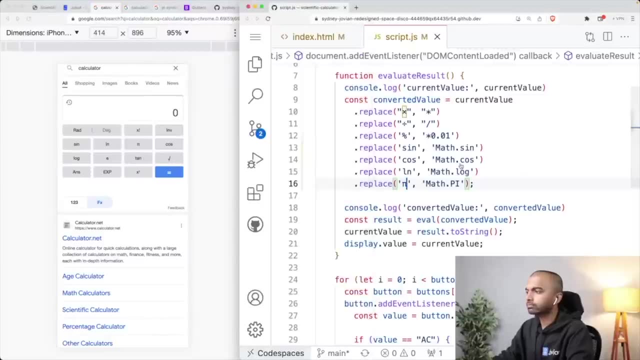 let's get one more line while we're. while we're doing this, This is interesting. Let's go ahead and implement one more line over here. Okay, we have log e, tan and square root. Fine, let's do it So. log, I believe, would be the log to the base 10.. And I can verify that by again going into: 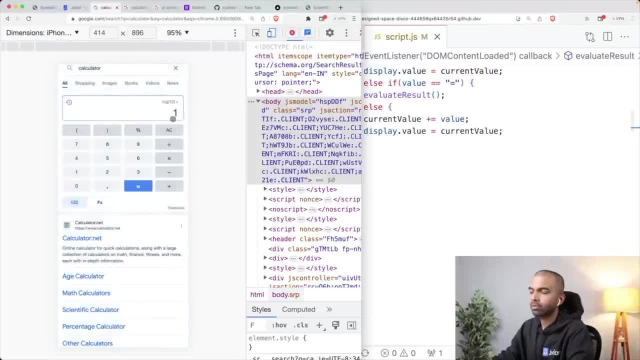 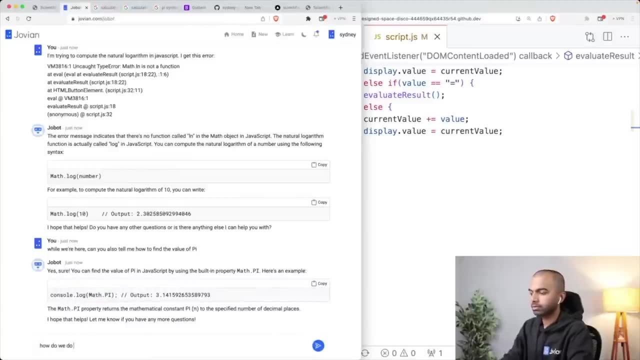 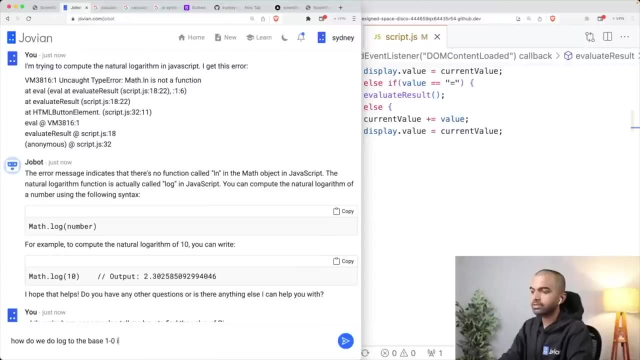 log to the base 10 equals one. Yeah, So log is log to the base 10.. So how do we do log base 10? Log to the base 10 in JavaScript? Yeah, I think it's gonna try and figure out. Yeah, okay, there's. 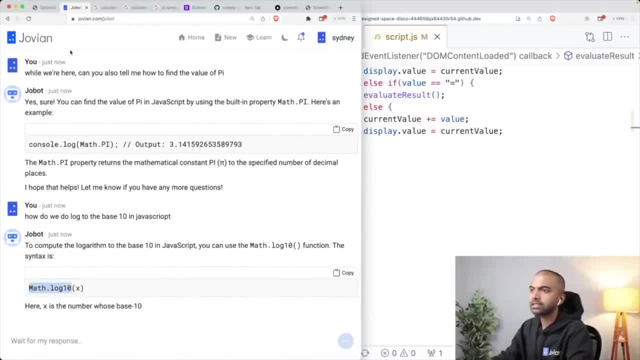 a math dot log 10x And that is going to do log to the base 10 for us. So we can do one more row And probably square root is going to be somewhat interesting. So let me just do one more row And 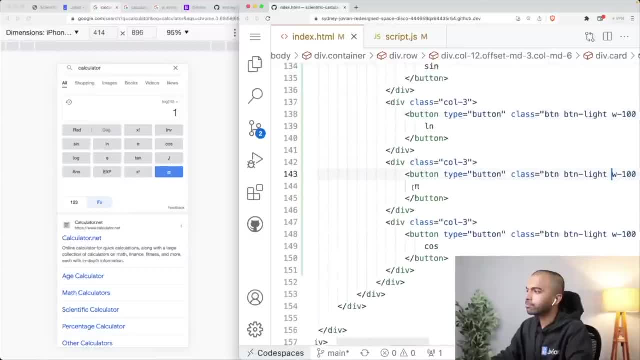 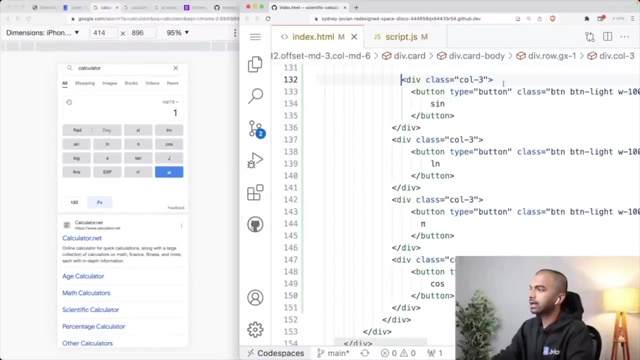 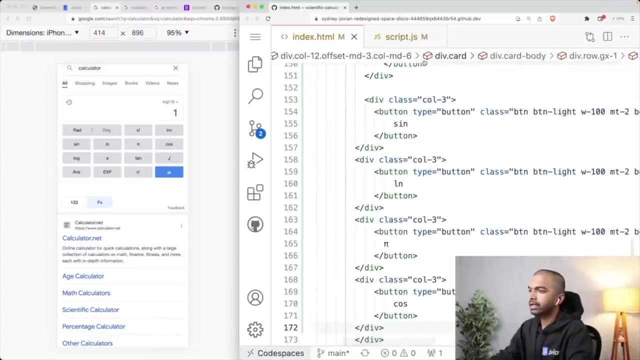 I'll leave the rest rest as an exercise for you, So that I don't give everything away. Let's see, So we have these buttons. I'm just going to grab these buttons once again And I am going to drop that in here. Let's add log. 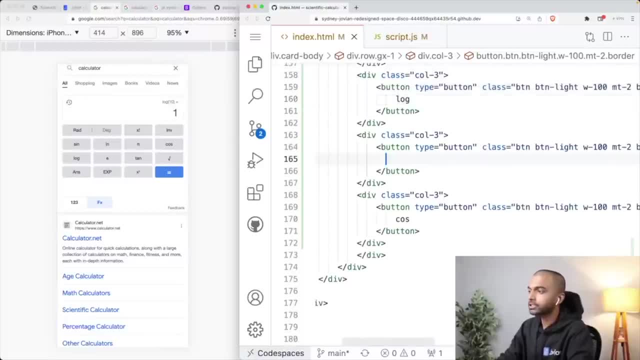 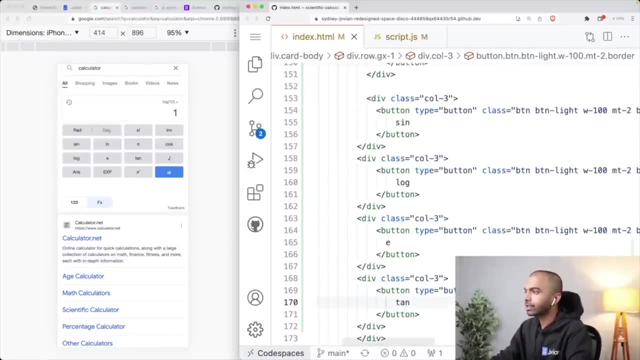 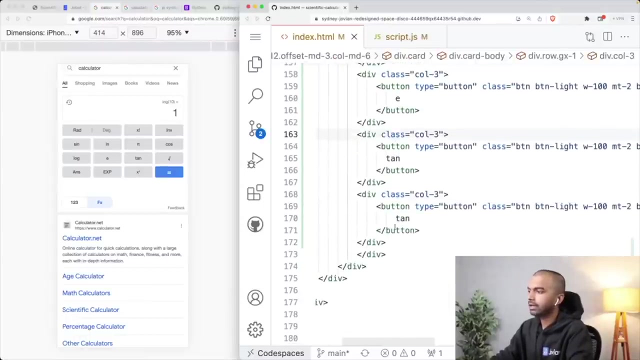 by the way, if you have any questions, please drop them in the comments. we will look at the questions And alongside, I want to tell you that wait till the end, because there's going to be something really interesting that you don't want to miss. Okay, so we have log e tan and the square. 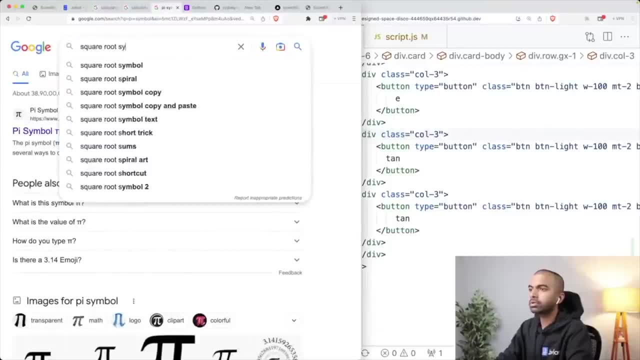 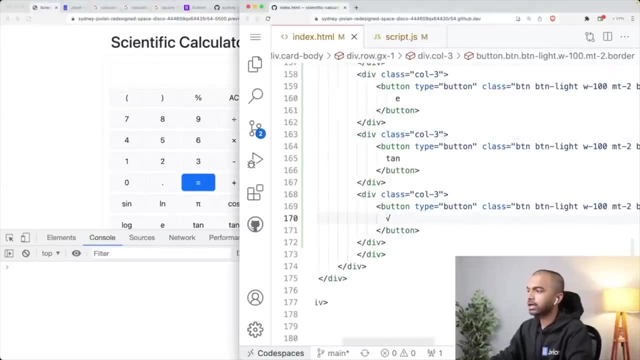 root symbol. So let's go in your square root symbol And let's grab that. Okay, that is called the radical symbol, But let's, Yeah, let's- just put that in here And now. we might want to just handle these as well. So what, what about? e let me just ask it. 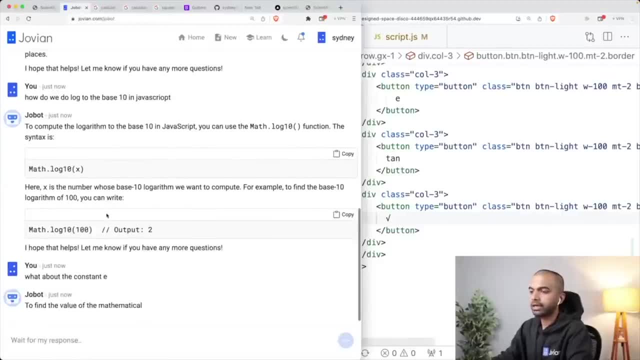 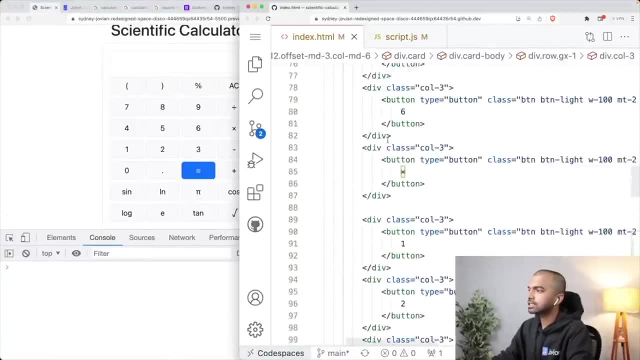 What about the constant e? How do I get that? Well, that is simply math: dot capital E. So we just use that. So let's go in, let's go into the settings, Let's go into the script or JS file. 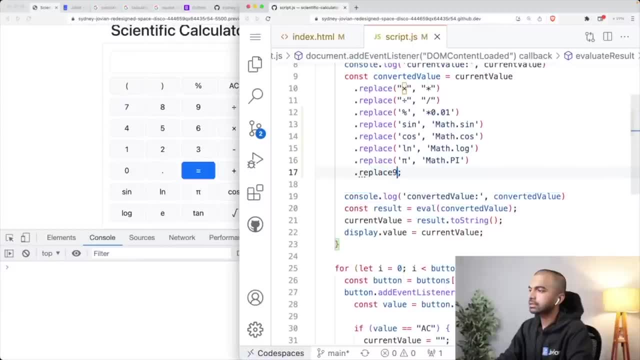 And let's add those replacements as well. So replace: we want to replace log with math dot log 10.. That's fine. We want to replace e with math dot e- Okay, and we want to replace tan with math dot tan before. 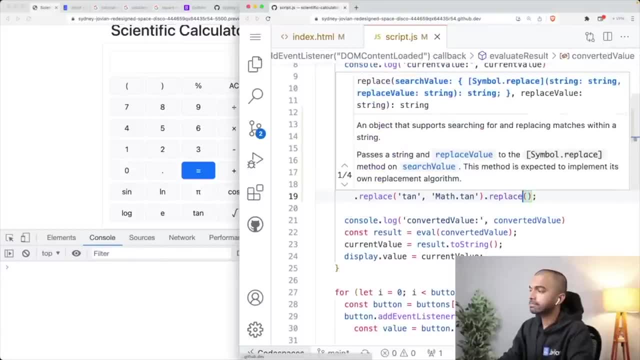 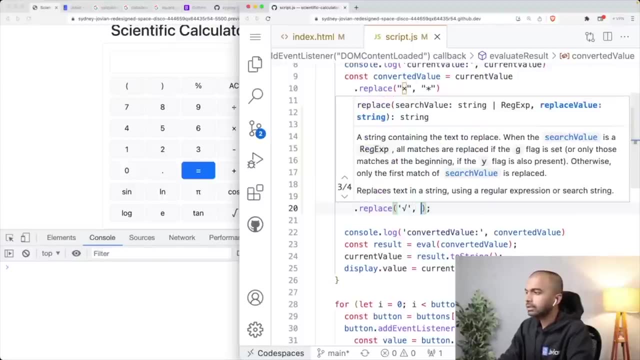 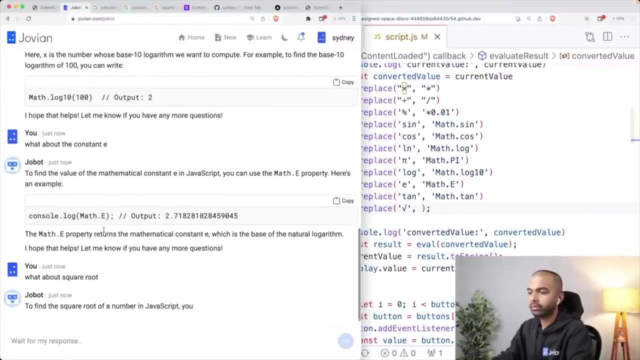 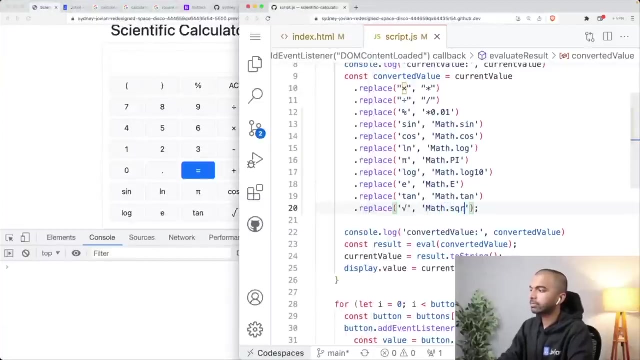 we actually evaluate it. And finally, we want to replace- let's see- the square root symbol. and what exactly do we replace it with? I'm not sure. Okay, let's just search here. What about square root? You just use math dot sqrt, So I'm just going to put in math dot sqrt right in here. Okay, 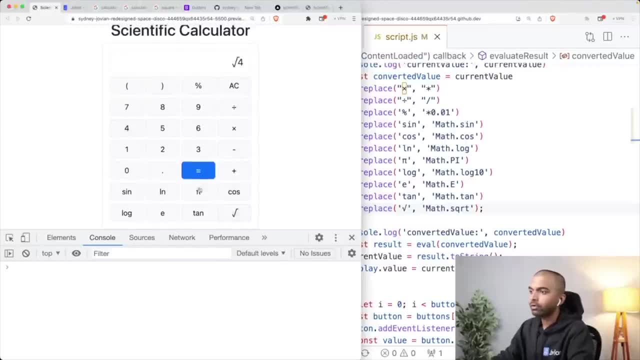 And with that, hopefully, let's see square root of four equals. Ah, okay, There's some. something went wrong here. I believe this requires a bracket, So I think we might need to actually put a bracket here. So square root bracket. 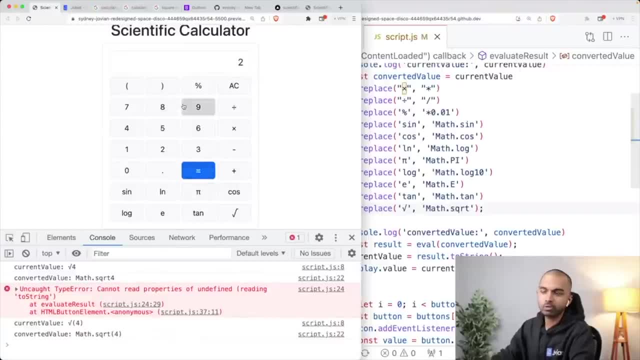 Four close bracket equals: Yeah, that's true, So that works. So we might need to be a little careful while working with square root, Or we might want to do something, and something a little more interesting while replacing, instead of just replacing the square root itself, Maybe. 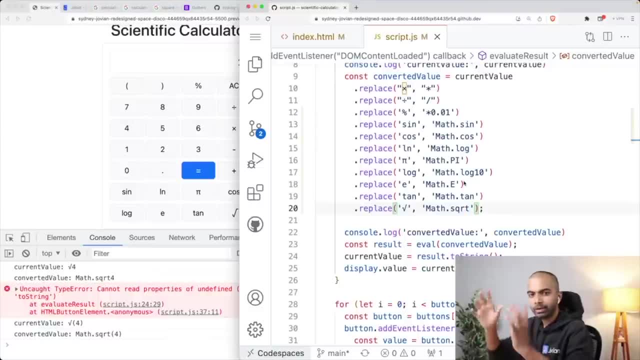 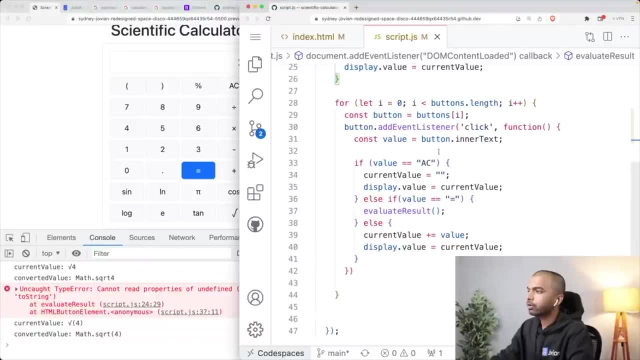 you want to take square root, followed by whatever comes after it, and put that in brackets or something. But for now it's fine. But another thing that I should do properly is I should maybe just put all of this into a try catch. Okay, so JavaScript has something whenever there's an. 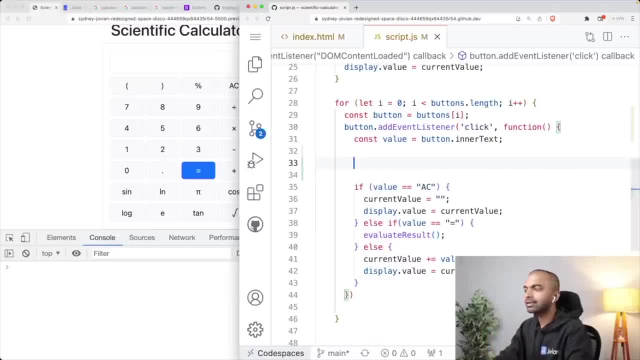 error. Okay. so JavaScript has something: whenever there's an error, you can actually catch the error and you can handle it in some fashion and maybe show a message to the user. So let's say try, And let's put all of this into a try block. Okay, so it's going to. 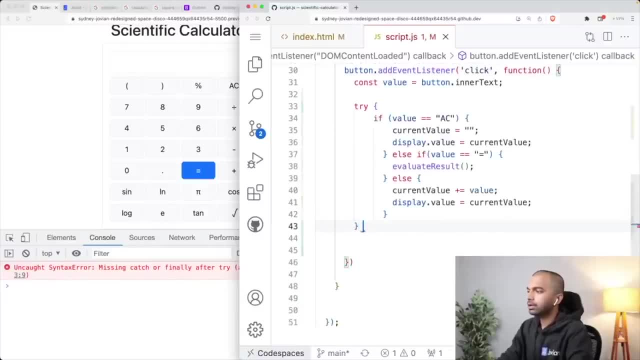 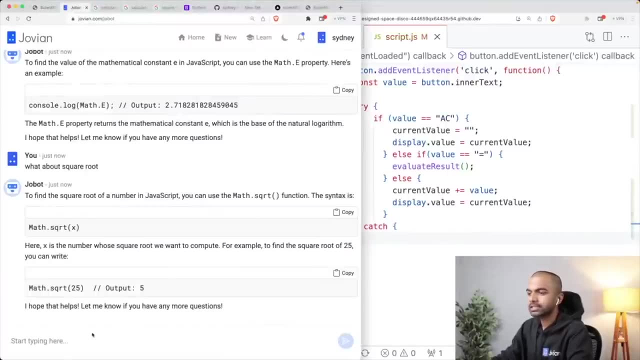 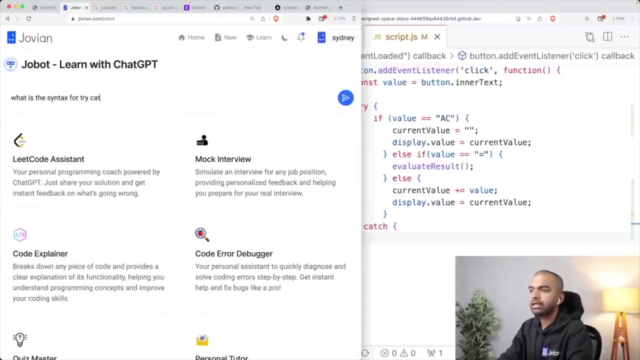 try to execute this code And if the, if, the, if the code works, then that's fine, But otherwise, okay, let me just search. what is the syntax for try catch in JavaScript? What is the syntax for try catch in JavaScript? Okay, the syntax is like this: So try, catch and then you catch an error. 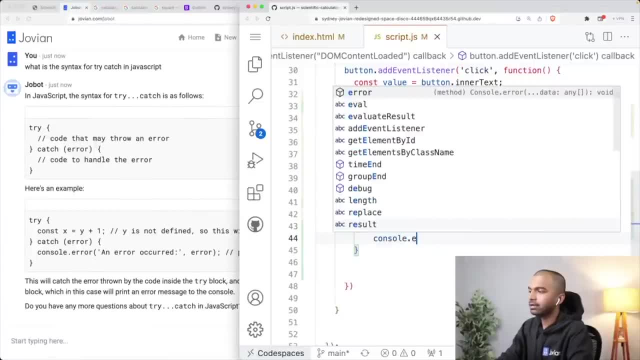 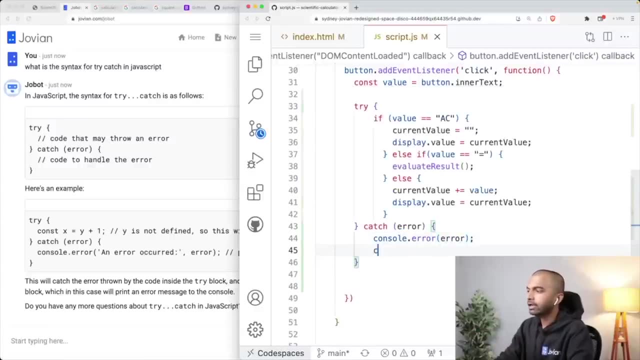 And then I'm going to print the error. So I'm going to say console dot error And that's going to print the error in that nice red format. So I don't want to get rid of the error. But what I can do is I can set current value equals error And I can say display dot. 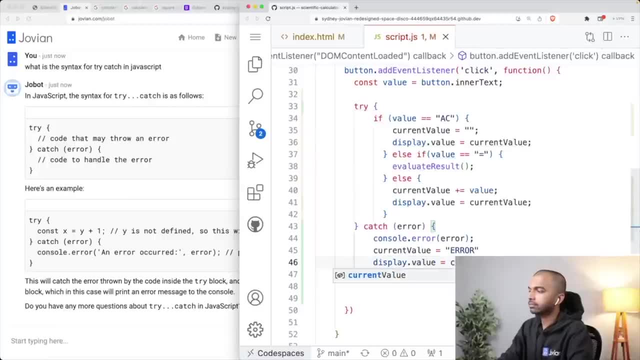 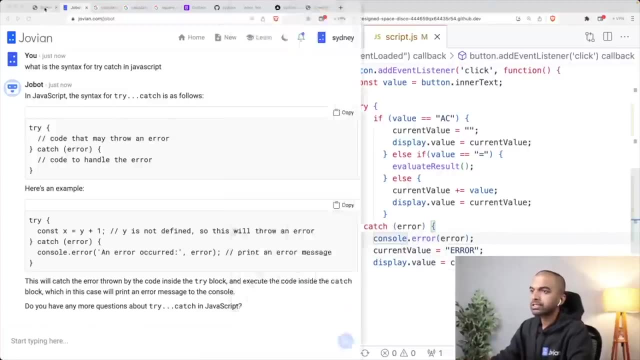 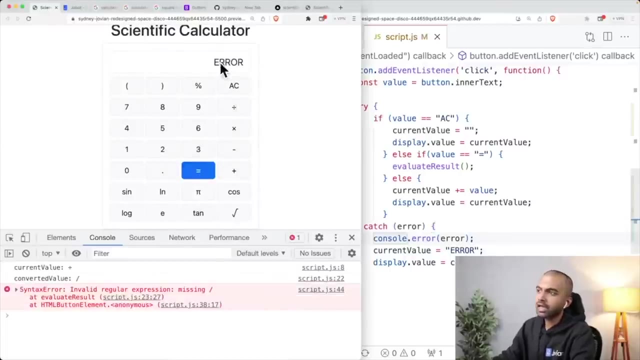 value equals current value. Okay, this way I'm also informing the user that there is an error And they can then deal with it somehow. Okay, so let's try that again. let's do something wrong, let's say percentage and let's do equal to here, And it just prints error over here, just like a. 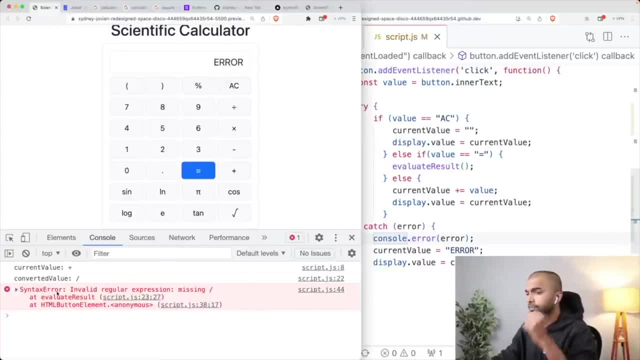 normal calculator And it also prints out the exact error for us, for the developer, to debug: invalid regular expression, missing slash or something like that, right, So definitely, this is something that you want to do, you want to try and catch these errors. So let's say you 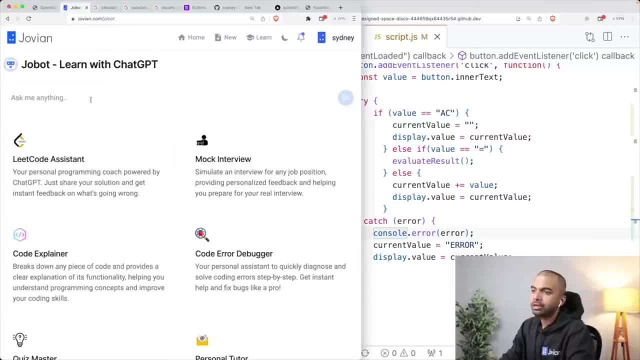 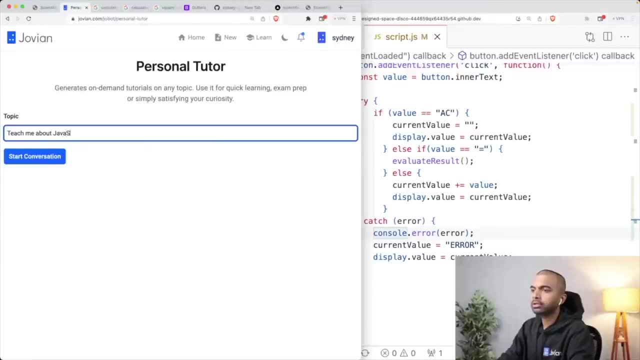 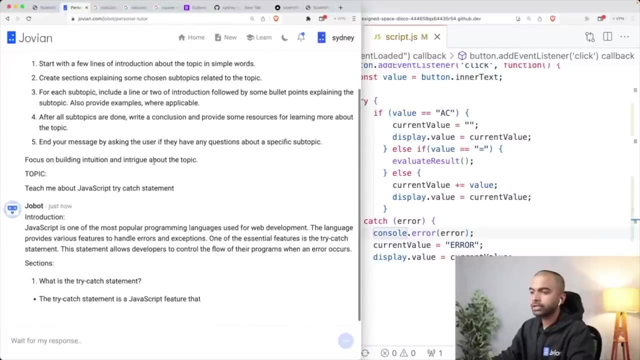 want to understand what exactly is try catch. you can actually ask your bot, or there's like a personal tutor here And you can just ask it: teach me about JavaScript, try catch statement and start conversation And it is going to just tell you a bunch of things about the try catch statement. Okay, what exactly does it's going? 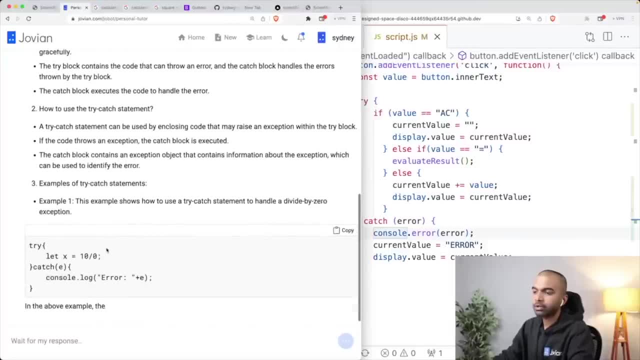 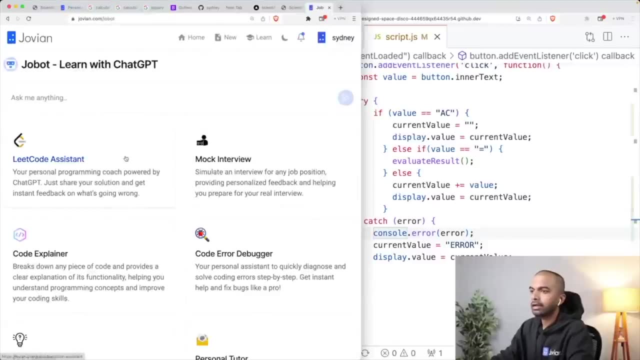 to maybe show you an example. So it's going to show you an example of how to use it, how to catch these errors, So you can generate tutorials on demand. just go on joviancom, slash, jobot, And if you want to use one of these specific tools over here, just scroll down and use them, or you can just 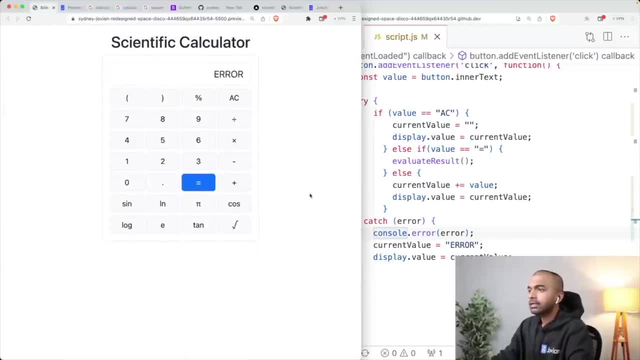 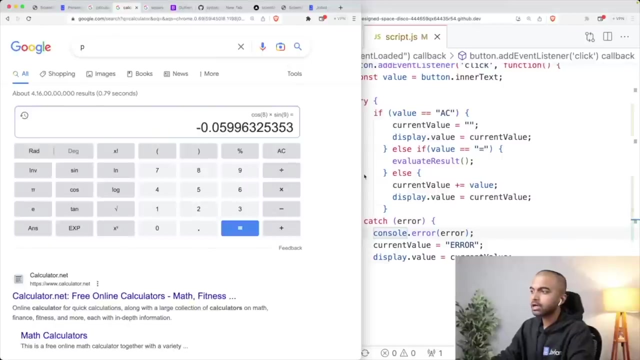 type, start typing and get help. Okay, All right, I think I'm pretty happy with the scientific calculator At this point. I am not going to go any further than this. I will leave the design, the responsive design, to you as an exercise. So how do you make it go from this? 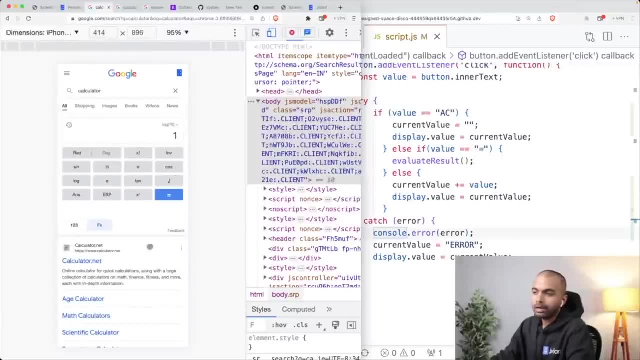 to this. That is something I'll let you figure out. If you can't, then just put all the buttons here below. that's perfectly fine. you don't have to exactly implement the design. And then there's also this, one other interesting thing that the Google, the Google calculator, does: you can. 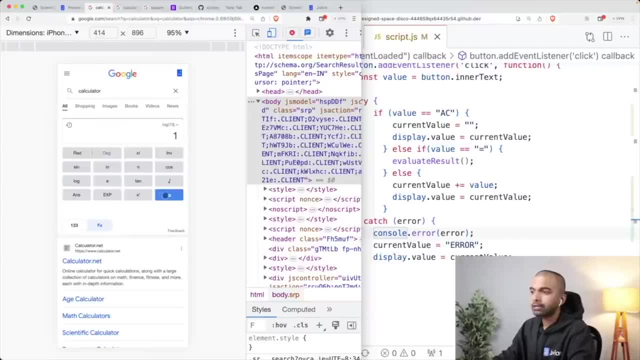 actually give it a certain input And when you click- when you click enter- it stores the previous result on top And you can see that pi equals is stored over here And it shows this recent history as well. that is probably too complex, But this is something might worth checking out. 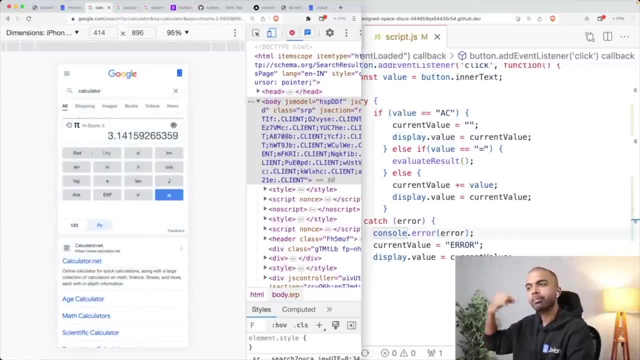 where you can have a previous result variable and just show the previous result, our Bob, the current result. Again, it's an optional part, So you don't actually have to implement the whole thing, But we've got ourselves a pretty good scientific calculator. I think I'm pretty happy. 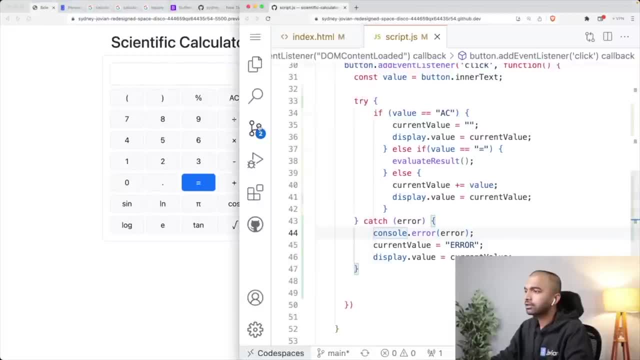 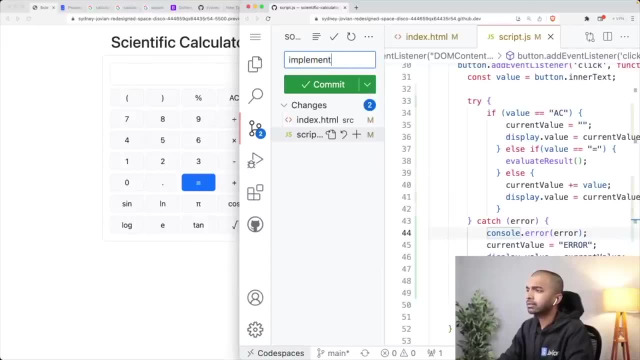 with this right now, So I'm just gonna save it over here. So let me go ahead and go ahead and say: implemented a few scientific functions. I'm just going to commit it and I'm going to publish it And my scientific calculator should now be live. Now, one of the things that 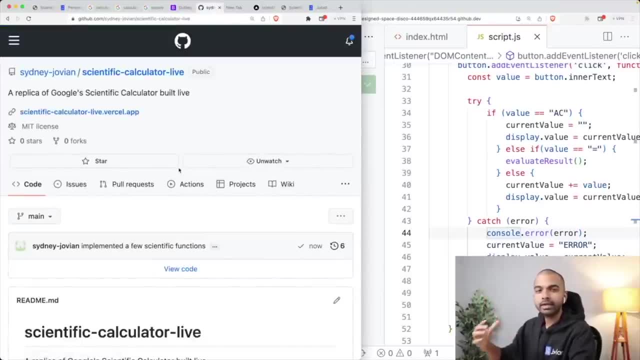 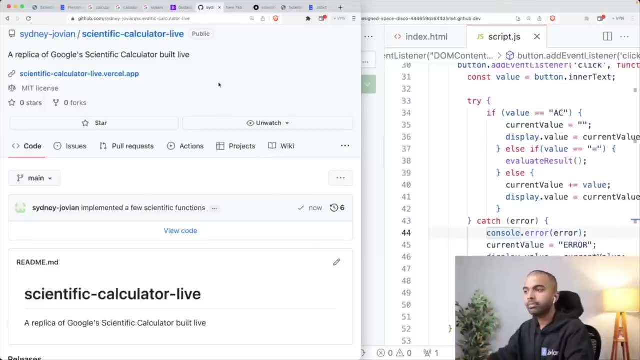 Vercel does the platform that we've used for deployment because it's connected to our GitHub. what it does is, every time you push to the main branch or the the main branch of the primary branch of the repository, it is automatically going to redeploy your 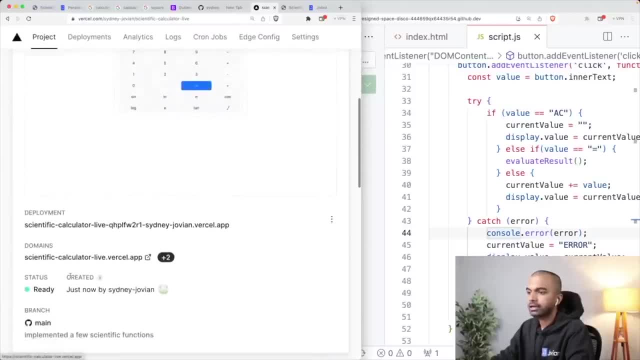 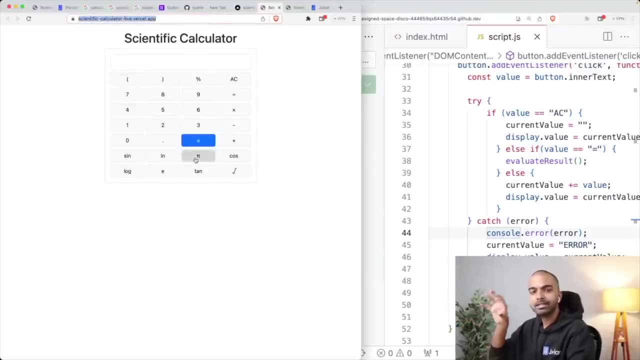 code And you can see here that now you can see that on my Vercel production website it is automatically now can. it automatically contains the updated code, So you can play along with it right now, And this is one of the best things with using an integrated platform like. 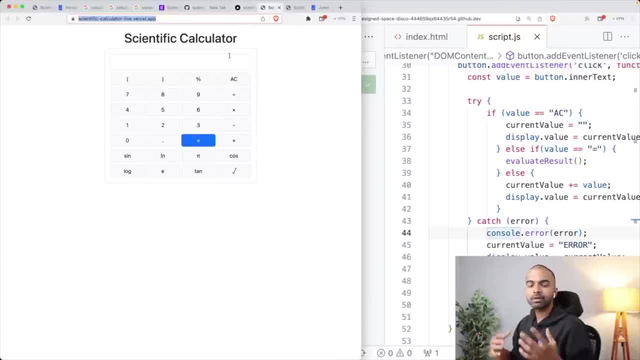 Vercel for deployment. Now you probably wondering: what if I make a mistake? Will that? what if the deployment fails? Well, it's going to use the previous version. But if you create a branch- and this is something that we covered when we talked about Git- but if you? 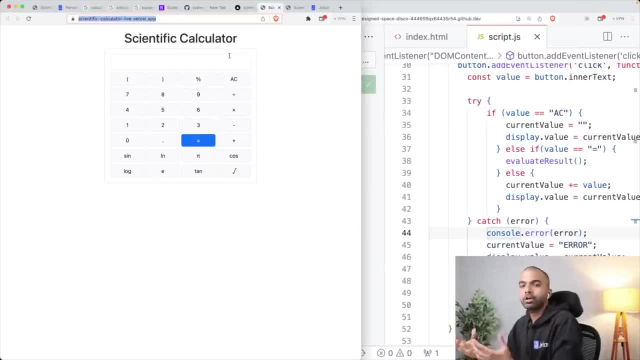 create a branch, then on that particular branch it's going to create a preview deployment- it's not going to affect your main deployment- And then you can create a pull request, merge it back. so that's all about the GitHub workflow. Okay, The final thing that I want to show you before. 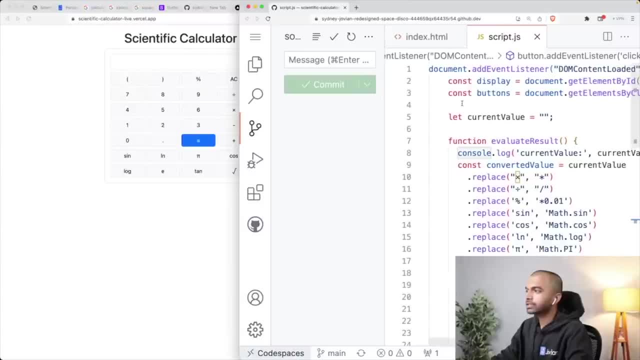 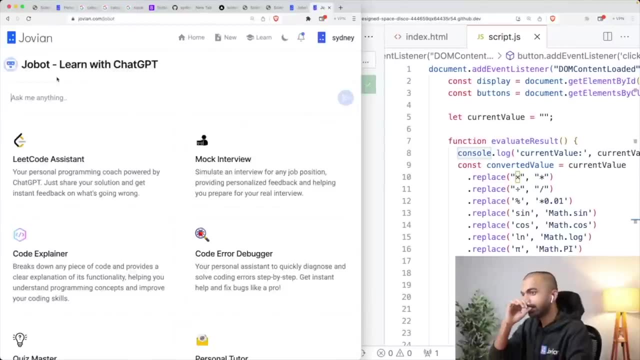 we close is that we didn't actually have to write any of this to begin with. the tools that we that are at our disposal are actually getting so good right now that you might not actually have to write in much of this code at all. So this is one thing that I tried to do earlier today. 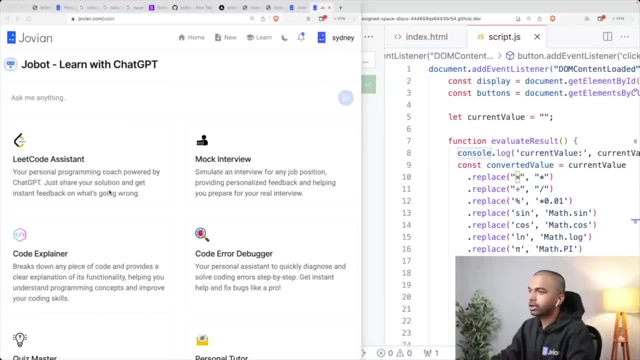 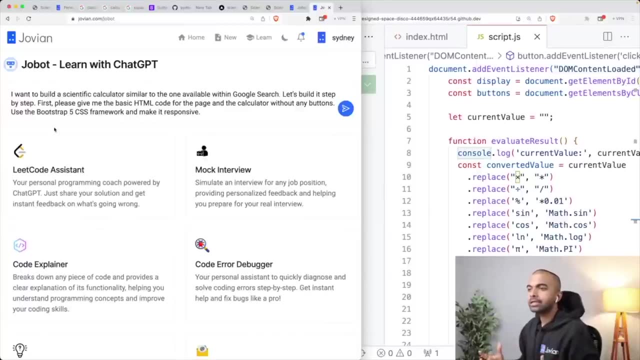 I just figured: what if I could just ask Joe Bort, just powered by chat, GPT, GPT 3.5 right now, soon GPT 4, what if I could just ask it that I want to build a scientific calculator similar to the one? 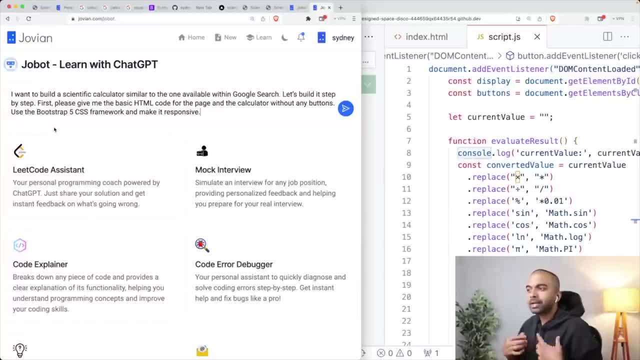 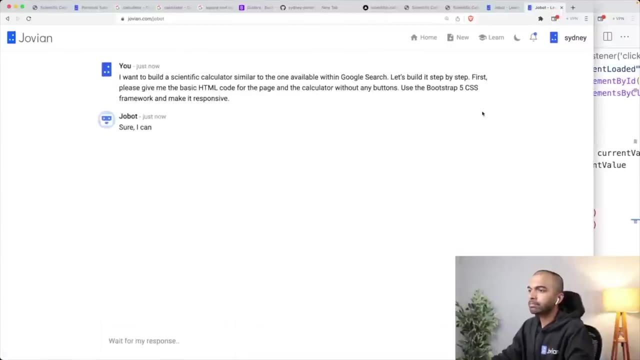 available within Google search. Okay, And let's build it step by step. So first, please give me the basic HTML code for the page and the calculator without any buttons, and use a bootstrap five CSS framework and make it responsive. Okay, That's what we've said here, And let's see if we 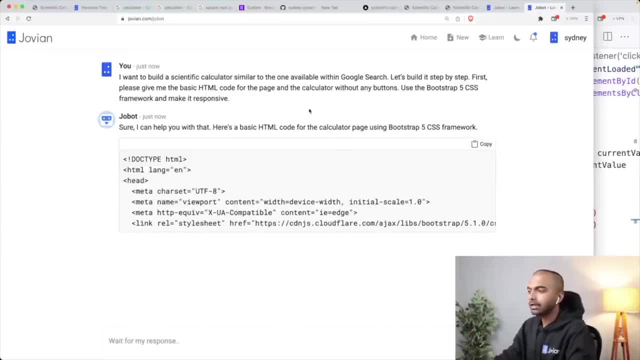 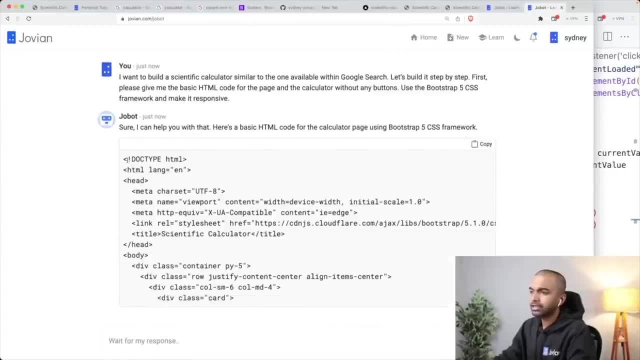 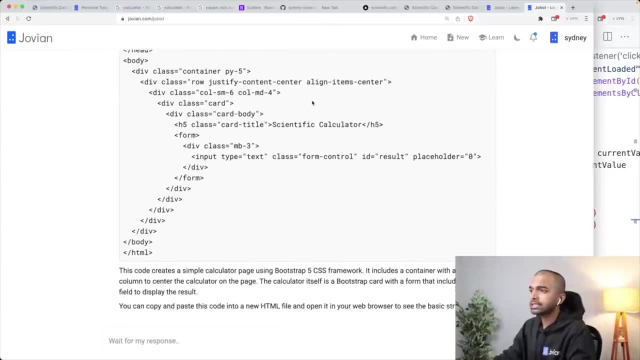 like it is okay, it's generating it. it created an HTML page for us. it has a meta, it has the right meta tags, it has this link tag for the style sheet. it has the scientific calculator and I've asked it not to put any buttons right now. 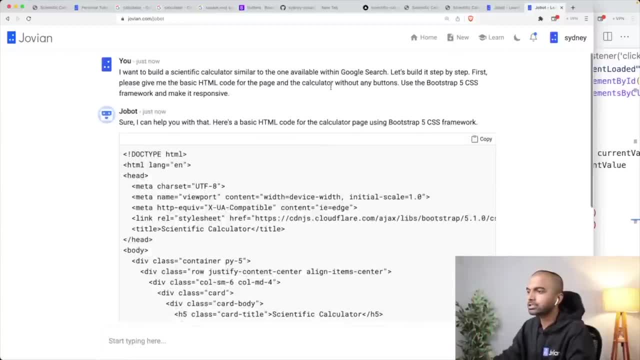 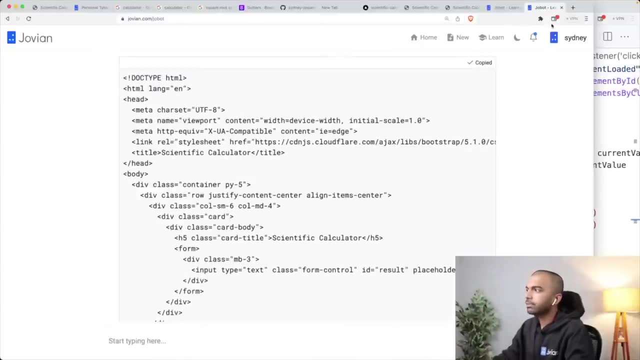 I'm going to add the buttons in the next step, but it could have just created the buttons for me as well. There's a limit to how many characters that can give you at once, And let me just grab this And let me open up this online platform where I can quickly test out HTML. 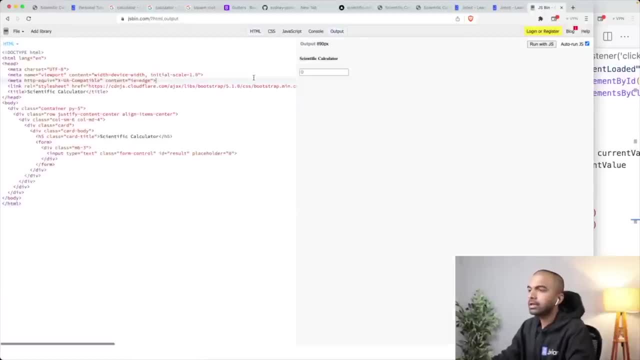 code. let me get rid of what they have here. let me put in this HTML- And you can see here that it is creating the scientific calculator- this basic layout already Now. the bootstrap styles did not get added And I have a sense of why. that is So one of the issues that the chatbots or the code 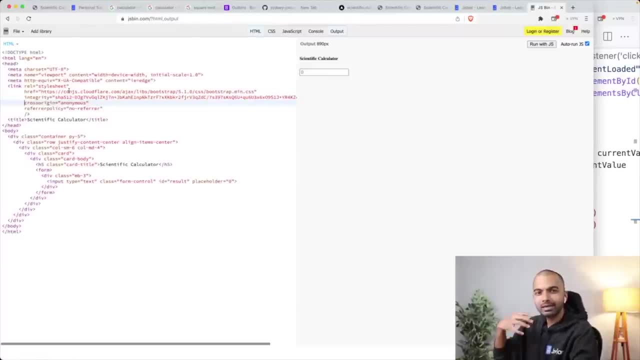 generation bots run into is that they may not, because they're characterized generators, they may not actually have picked up the right integrity, which is the hash that is used to verify the link tag. So you might need to replace the link tag. So you might need to replace the link tag. 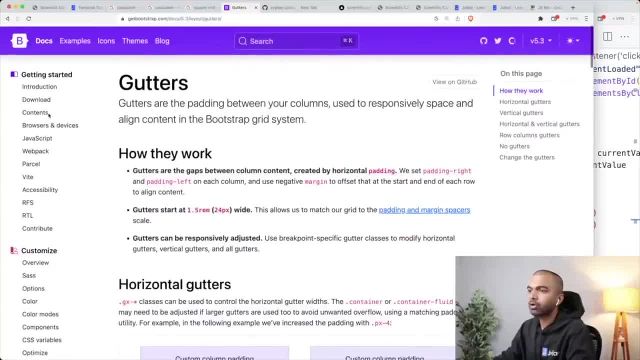 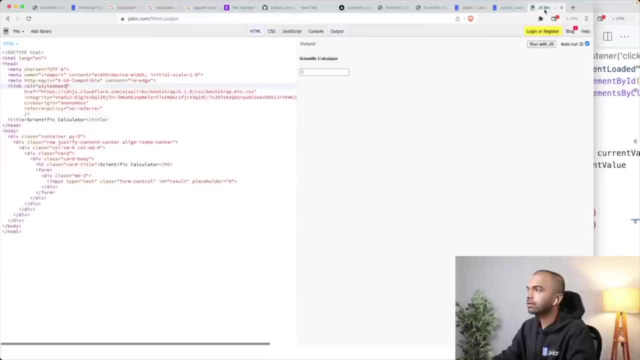 So you might need to replace the link tag with the actual link tag from bootstrap. So I'm just going to go back in here, go into introduction and grab the link tag from bootstrap itself. Okay, so let's go in and fix the link tag. So you should always verify any AI generated code that. 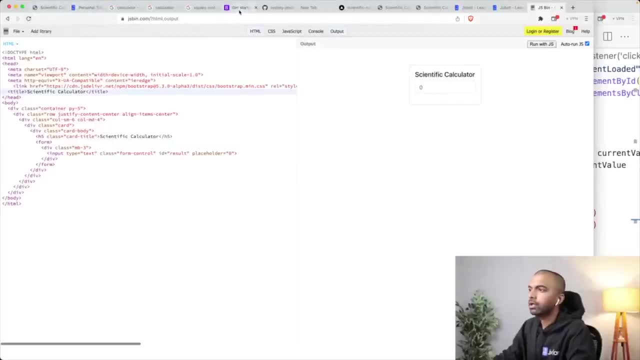 you are working with, you should always go through every line of code. But just because it's not directly giving you the result that you want doesn't mean that it's not going to be able to solve your problem. Okay, let me add that script tag in here as well, So it is created for me, the 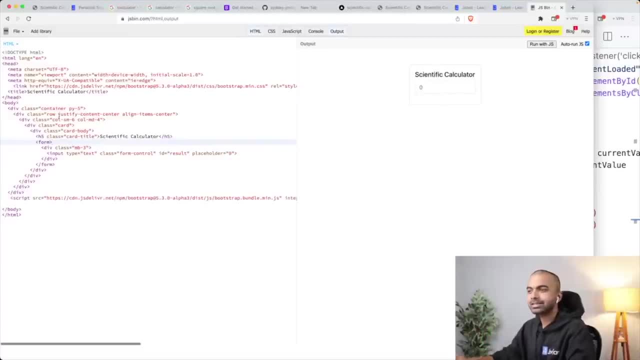 scientific calculator. So I'm just going to go back in here, go into introduction and grab the link tag And you can see that it's followed the same best practice that I followed, or maybe I copied it, But you can see that it has this row over here And it has this column And okay, it's made. 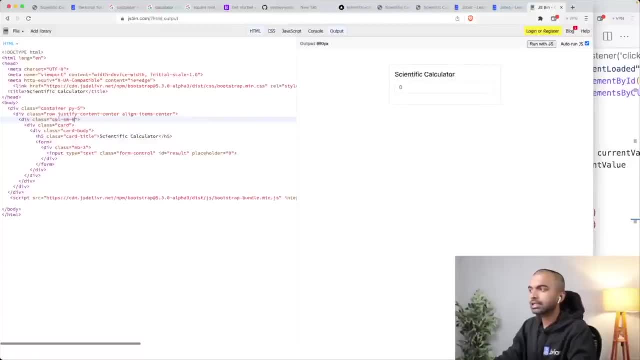 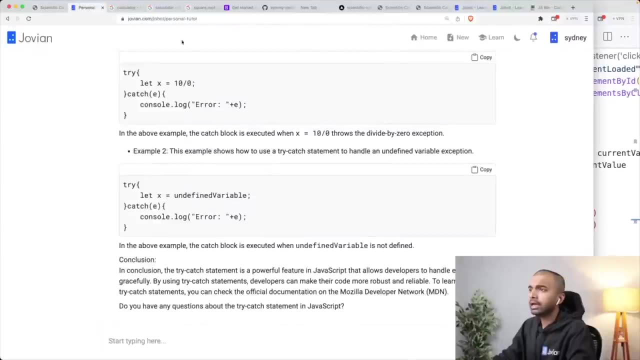 this calculator too narrow, So I'm just going to stick with: call MD six or call SM six. So so far so good. Okay, let me now go in here and let me come back. Okay, so now let me ask it. Okay, give. 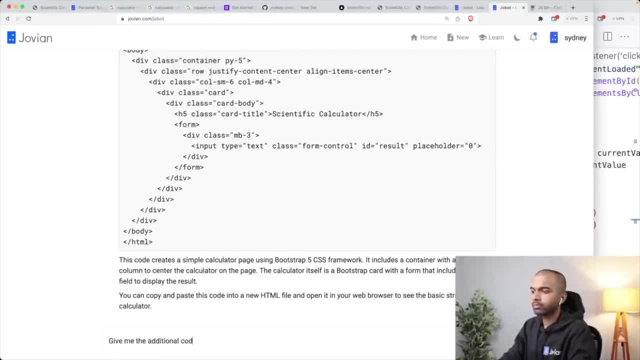 me the additional code To add the buttons within the calculator And I'm just going to tell it not to don't rewrite the entire HTML. Yeah, and let's see if it can just give me the code to add the buttons And it. 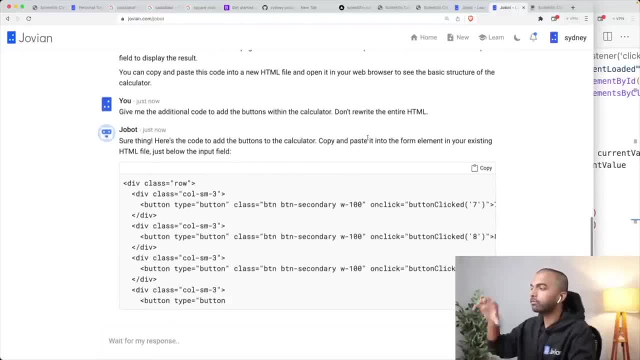 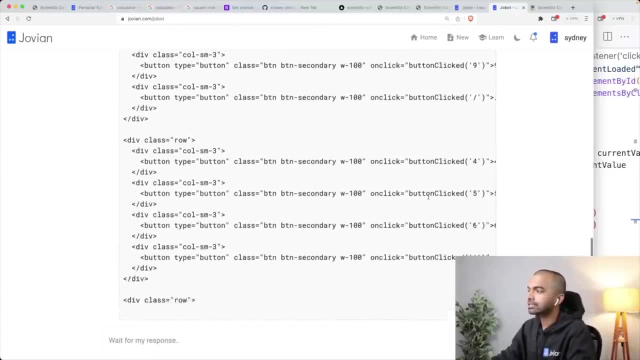 does So. now it tells me that copy paste this code into the form element just below the input field. So let's do that. So now it's adding a bunch of buttons. you can see it's adding 789, slash, 456, star or 123.. So it probably also. 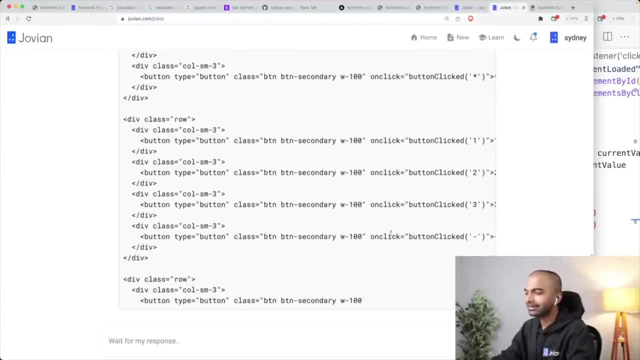 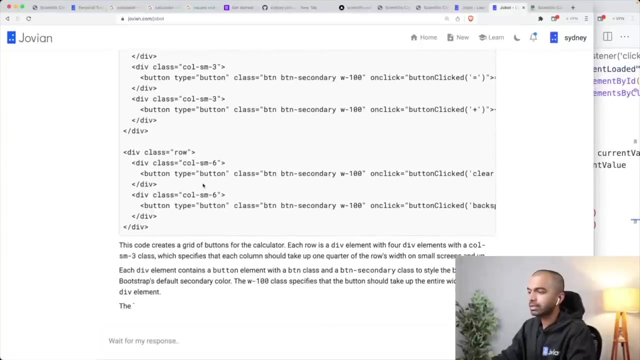 knows what Google's calculator looks like or a calculator in general, And that's great, And it's got these bunch of other buttons here at the end, equal to zero dot, And then it's got maybe a button called clear, That's like a huge button, and maybe a backspace button. Okay, And it's given me. 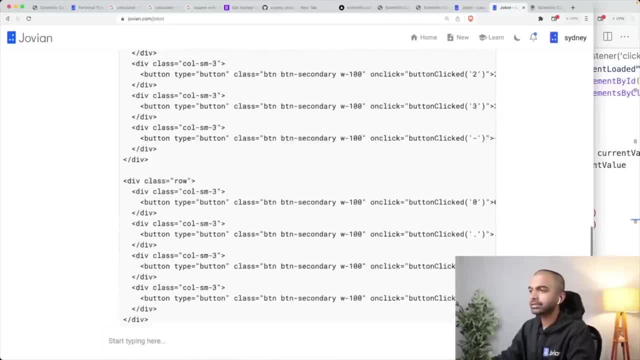 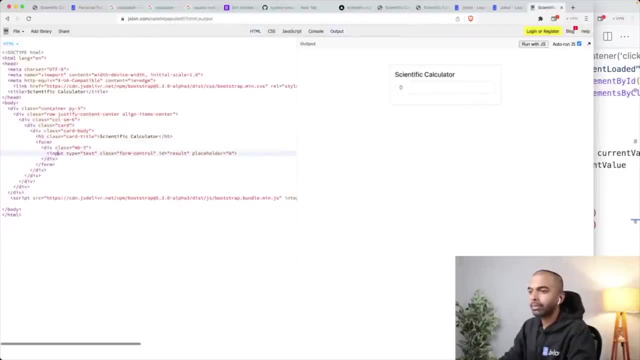 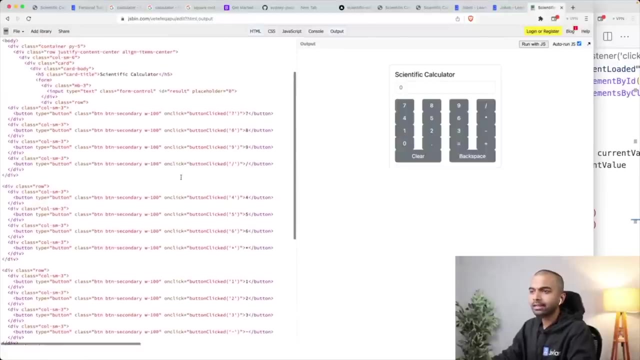 some explanation about the code as well. Yeah, this is just insane. I did not expect that things would get to this point, But it is, And let's just put that in here. Let's add in the buttons, Okay. well, it's not looking too bad. I think definitely. there's maybe some layout changes. we 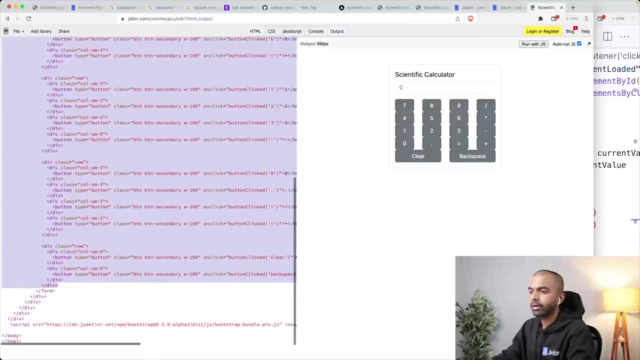 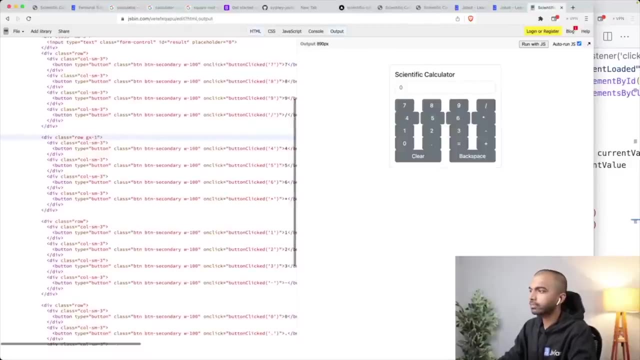 may have to do to make the buttons look slightly nicer, But I'm not complaining. I think this is fine for now And we could, for example, go in here and we could say gx one, right, Not just for this row, but for every row. So we could go in and say gx one over here. 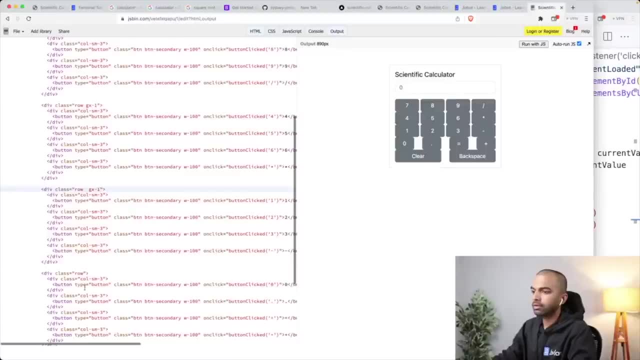 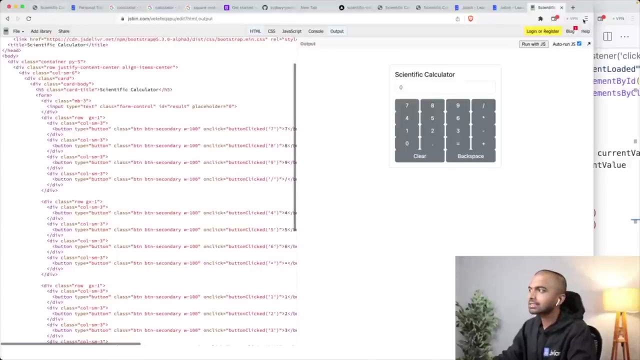 we could go in and say gx one over here, And we could go in and say gx one over here And maybe gx one over here, And of course it is using button secondary. maybe we could just fix that and use button outline. And let me just actually ask it if it can add some space between: 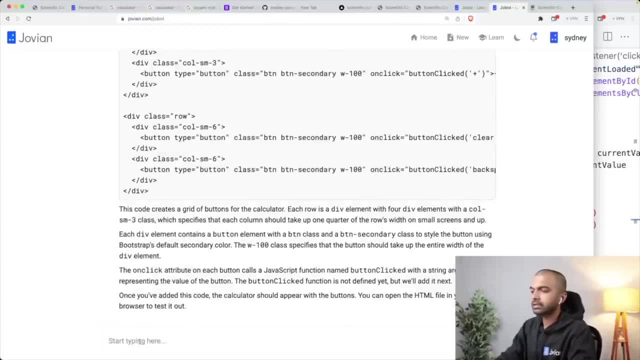 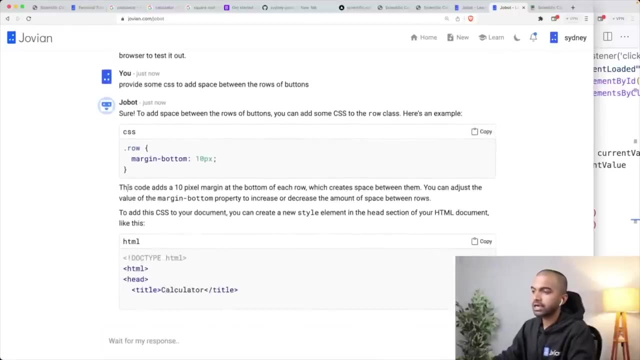 the buttons. So let's say, provide some CSS to add space between the rows of buttons, Okay. So now it says, okay, just add that. That's it, just add the margin And you can just add it within the. you can just add it as a style. 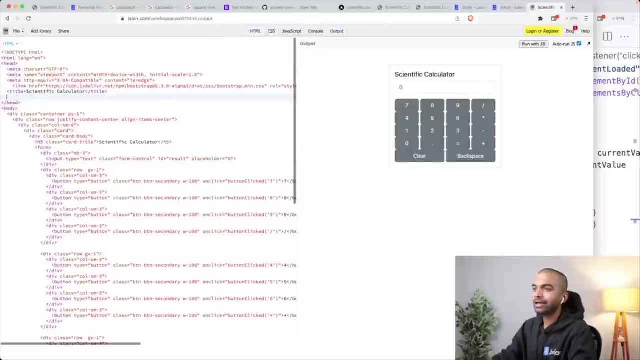 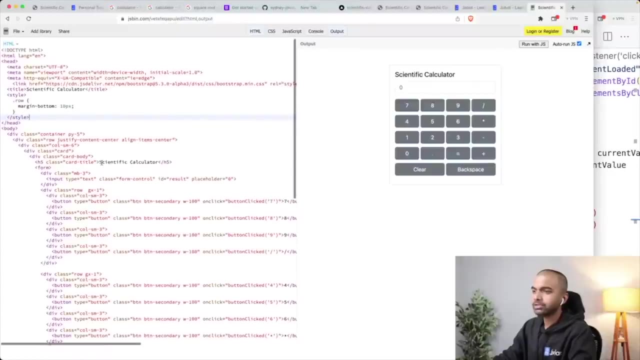 tag within your HTML And I just go in there And I just put that in there And there you go, the scientific calculator is looking rather nice. I could maybe come in here, maybe the H5, maybe just text centered, And I could maybe just make it read only: Okay, that's nice, And but it. 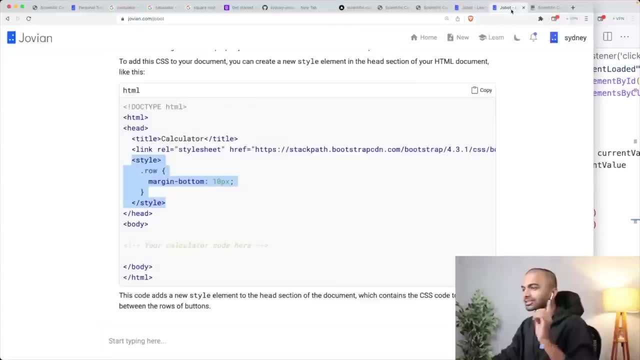 of course, doesn't have any logic yet. Let's see if jobot can actually write the logic. Okay, this part I'm not too sure, But can you now write the logic for the buttons using java script frameworks, because sometimes it might use jQuery or something like that? 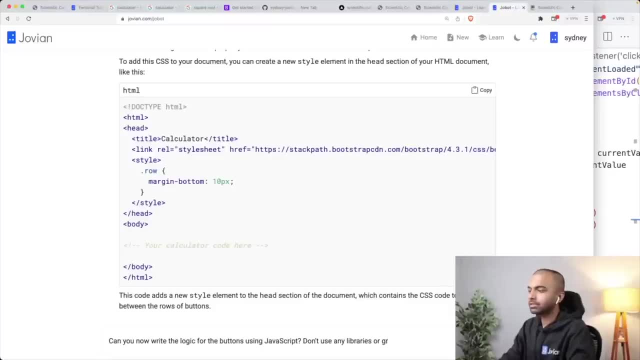 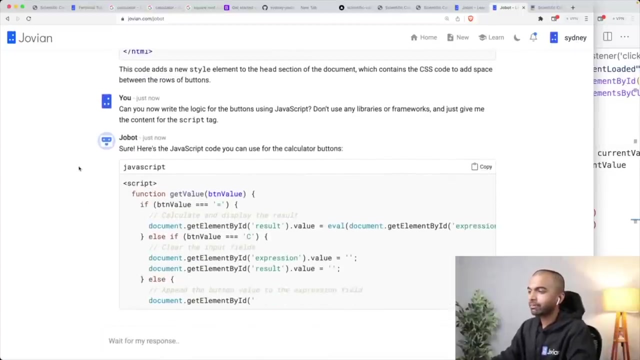 That's what a lot of examples on the internet contain. Don't use any libraries or frameworks and just give me the content for the script tag. Okay, And let's ask it and let's see if it can do that. Okay, Perfect. 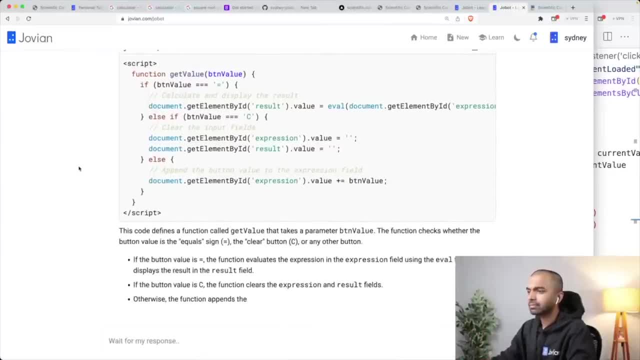 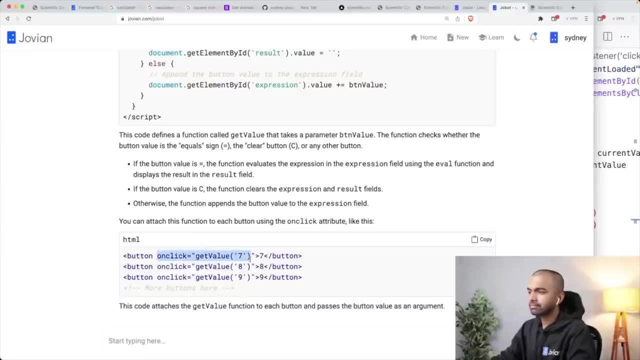 So it's giving us: Okay, it seems like. then I then have to add this: Okay, I let me tell it I don't want to add, I don't want to add any on click handlers. So you can actually tell it that you're not happy with the code. 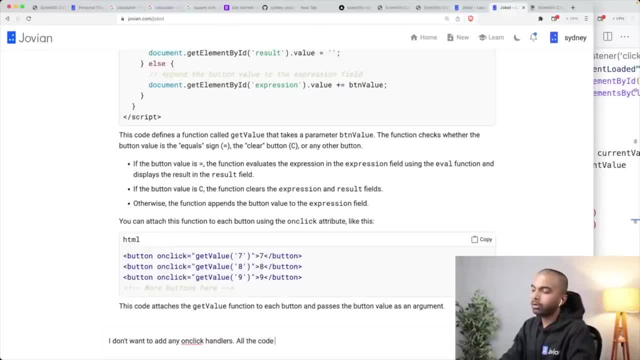 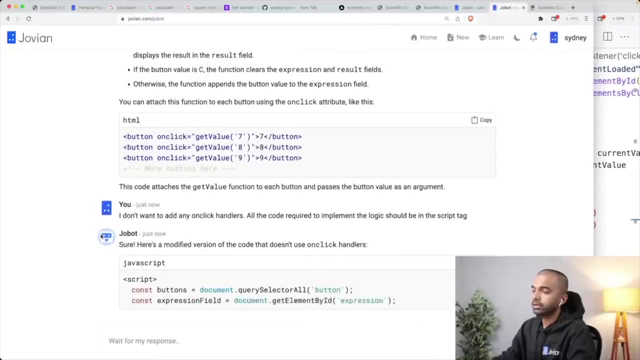 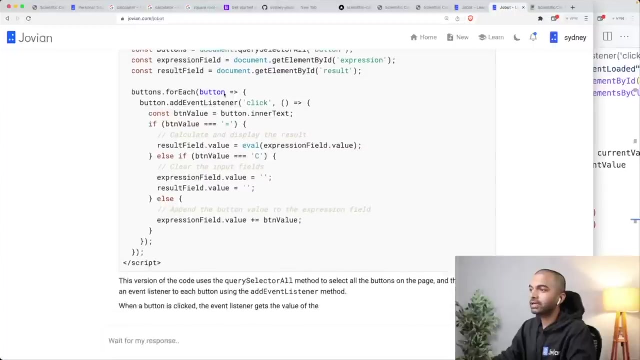 I don't add any. on click handlers. all the code required to implement the logic It should be in the script tag. Okay, Yeah, look at that. So now it's just doing document dot query selector, all expression field and it's given. 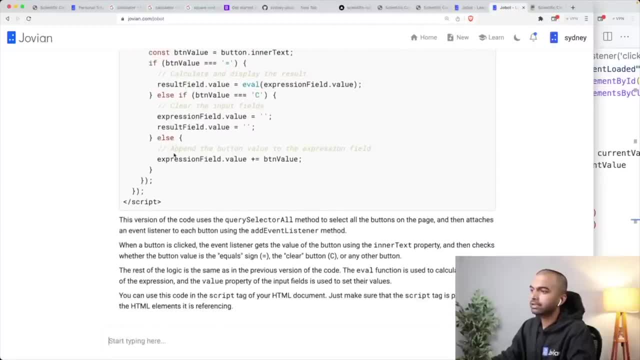 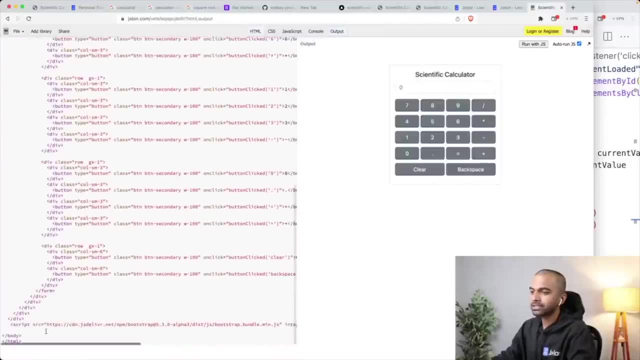 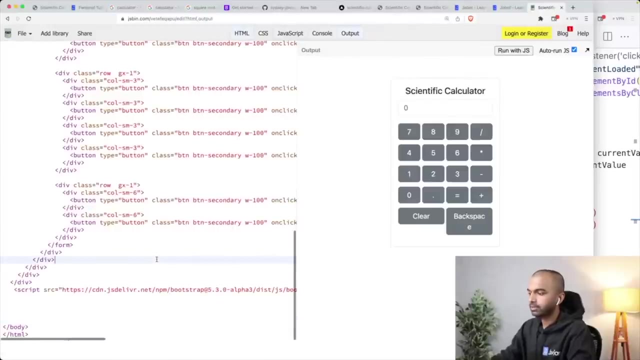 it's given it the type ID expression, probably, and then it is evaluating a bunch of things. Let's see. Let's just copy this JavaScript and let's see if that works. I am not very confident that this is going to work. GPT-4 would definitely do a much better job. GPT-4 is the newer version of chat GPT. 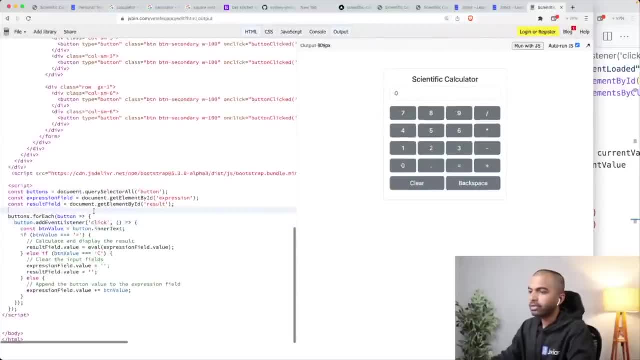 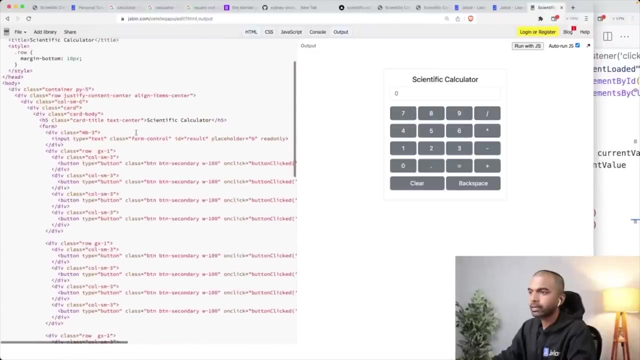 But okay, Yep. So now we have added some event listeners. I think we might want to put it inside document dot element ready or something like that. But let's see if this works. Seven, Nope, Let's see. So what does it say? the expression field is called. 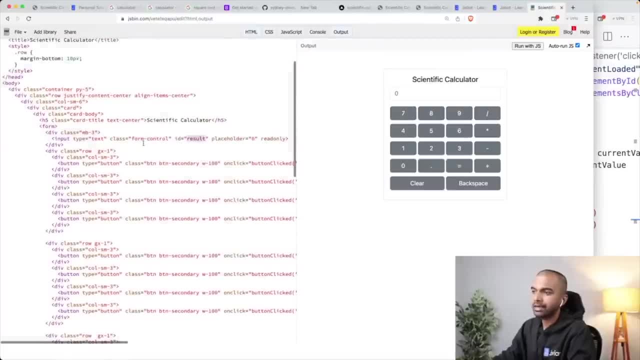 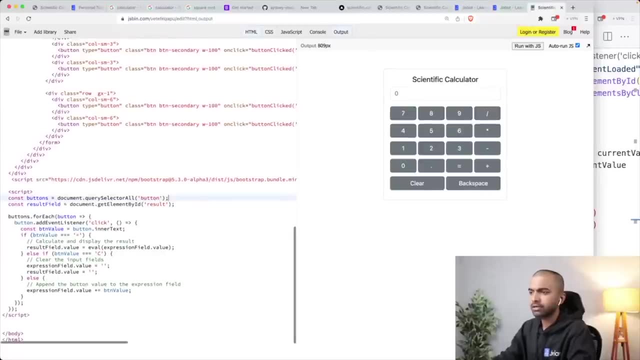 Okay, the input does not. input has the ID, The ID result. So maybe this should be: get element by ID result. What's the expression field? Well, there's no expression field, Maybe not. Maybe this is you've added the result field. 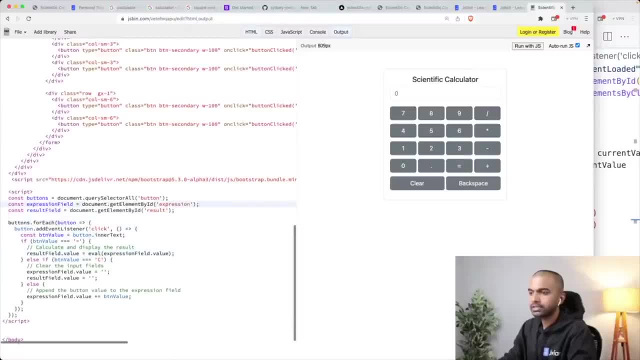 Okay, Let's just do, Let's just change that to current value. Well, what if we just give it the ID result As well? so looks like it is it has two fields: one for expression, one for result. maybe it got confused there. 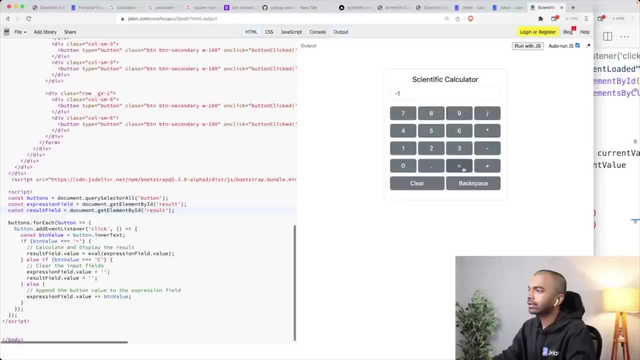 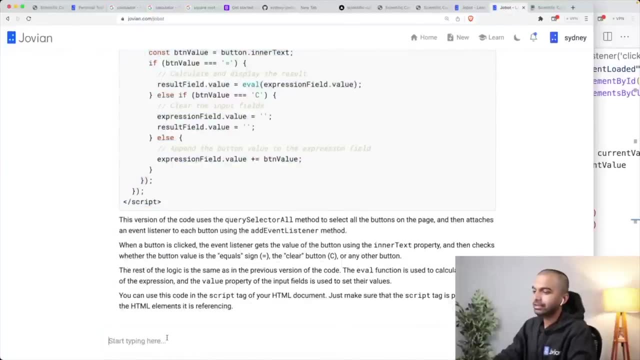 But look at that. eight minus nine equals minus one. That's not bad. Okay, clear and backspace are not working, So let's tell it. you're not handling the clear and backspace buttons. Please update the code. Also, there's no field with the ID. 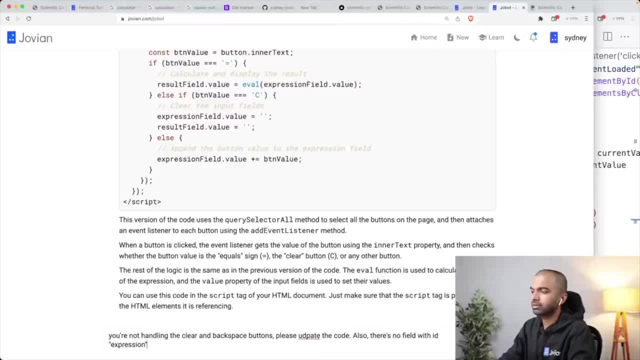 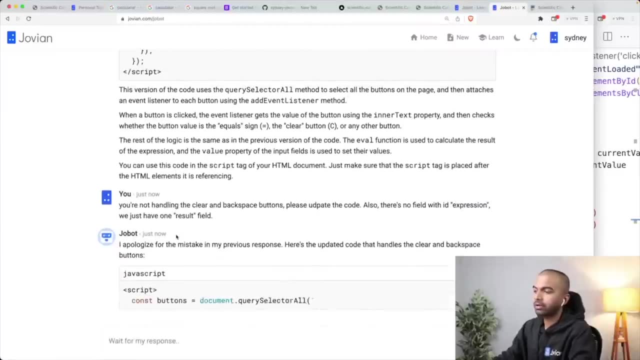 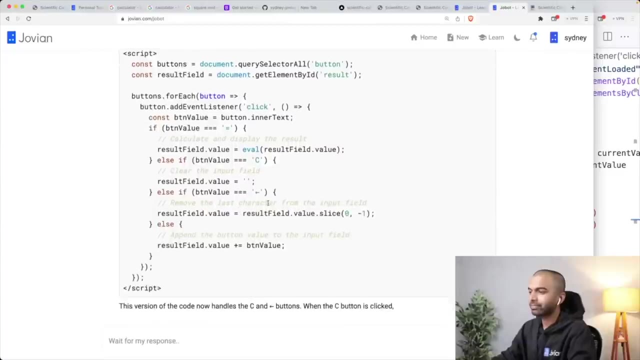 Expression. We just have one result field. Okay, it apologizes for the mistake, obviously, And now it is going to update things to also handle the Yeah again. it probably mess things up a little bit, like it is thinking about C and slash. I guess it probably doesn't have. 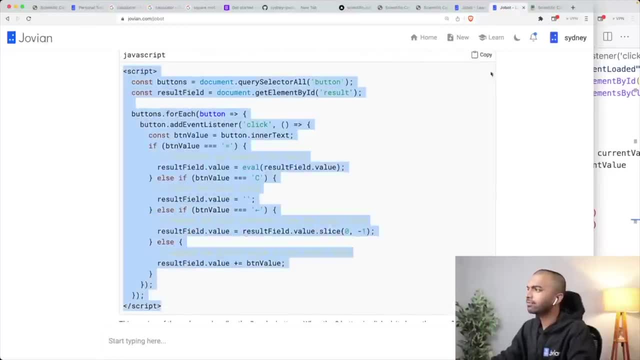 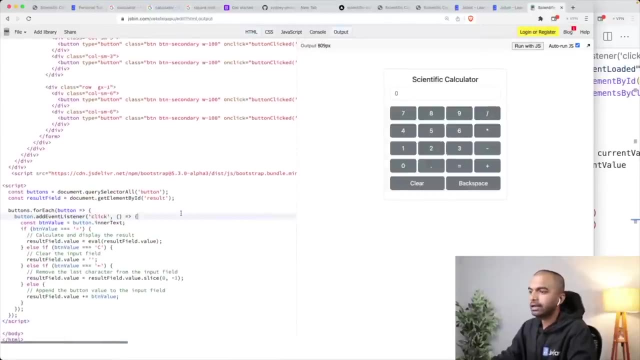 the full context with it anymore, But let's go ahead and fix, make that small fix. This is still a lot faster than coding everything from scratch, Of course, And yeah, so here it's using this backspace buttons instead of the back word backspace. 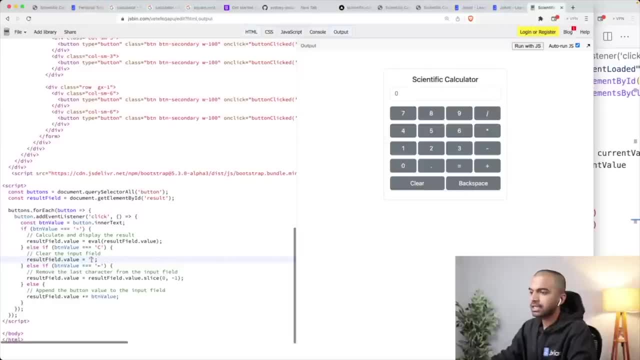 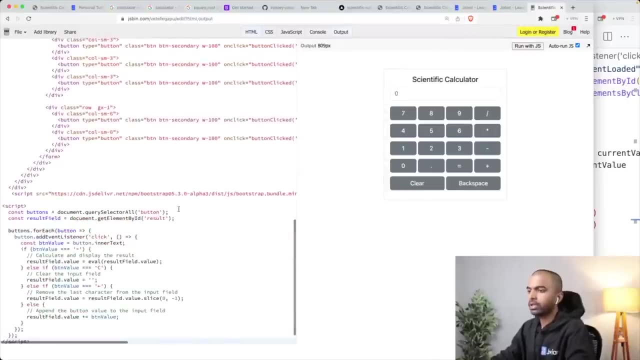 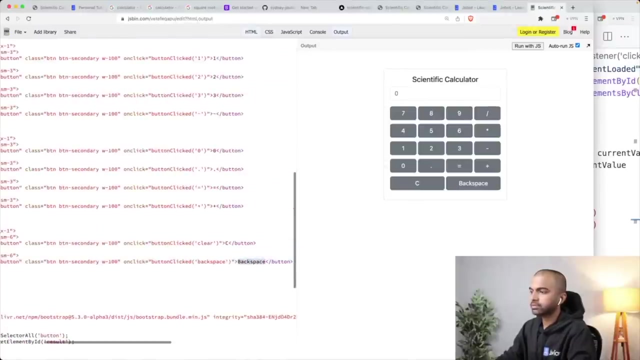 It's using this, this arrow, and it's using C, So maybe just let's replace that with clear And let's replace that with: or how about we do the other thing? we, we replace clear with C and and we replace backspace with the arrow character. 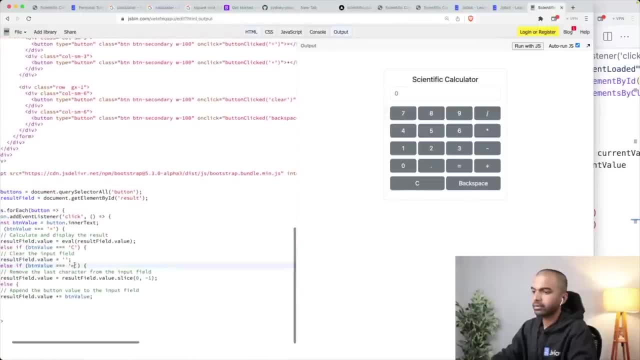 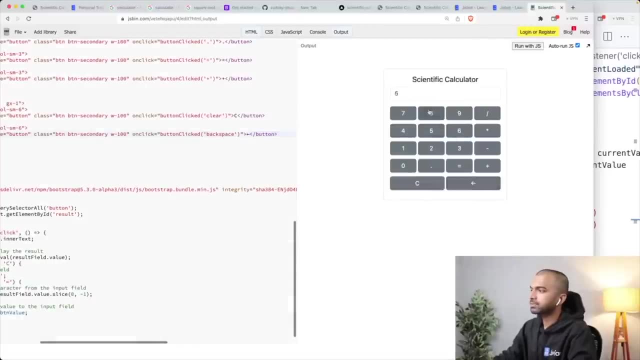 Okay, Okay. So how about that 56 and that backspace is now working. and 56 589 times 23 equals 13457.. Yeah, 580 89 times 23.. That's actually right, Great. You could probably also now go in and say add sign log and a bunch of other buttons. 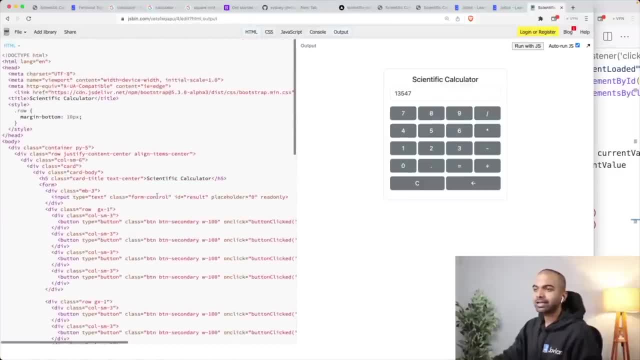 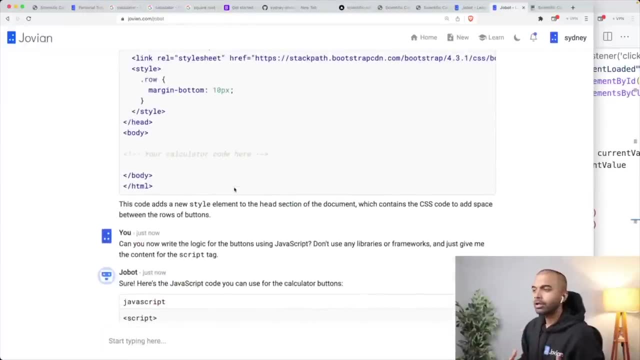 But I'm pretty happy with this. It just generated. It generated an entire scientific calculator with maybe two or three messages. It is just insane. And not only that, it also we also just copy pasted a bunch of errors that we encountered. 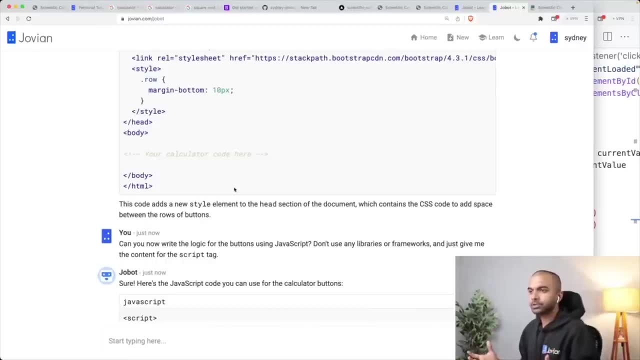 And it's all those errors for us. So use these tools, use chat, GPT, use jobot. Of course, verify the code that it writes. do not just depend on the code without verification. I've not had a chance here to look through every line of code. 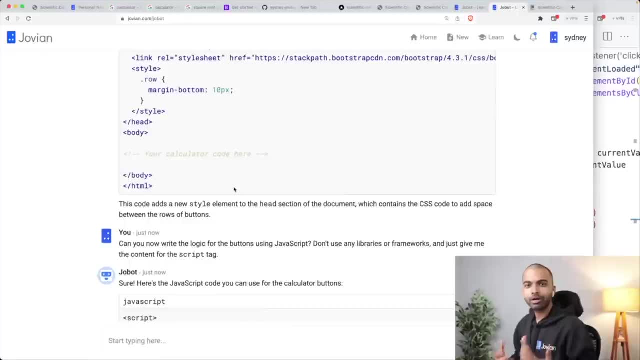 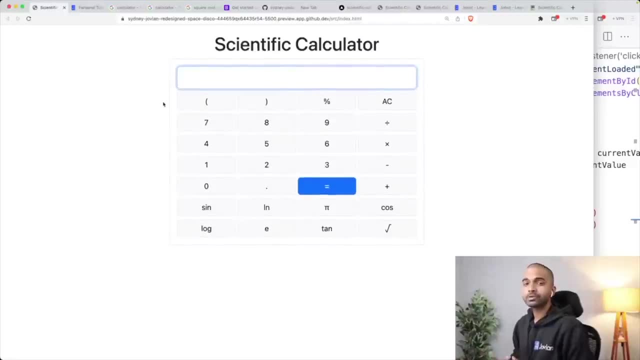 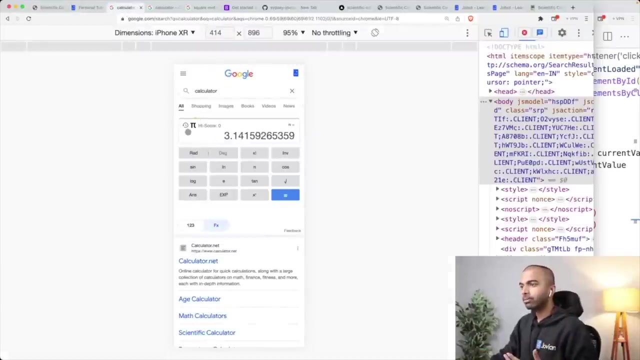 But you should. you should do that Because it may introduce some security vulnerabilities or something like that, But in any case, that is how you build a scientific calculator using HTML, CSS and JavaScript. I hope this was an informative session. A lot of things that look fairly complex are actually really simple to build out. 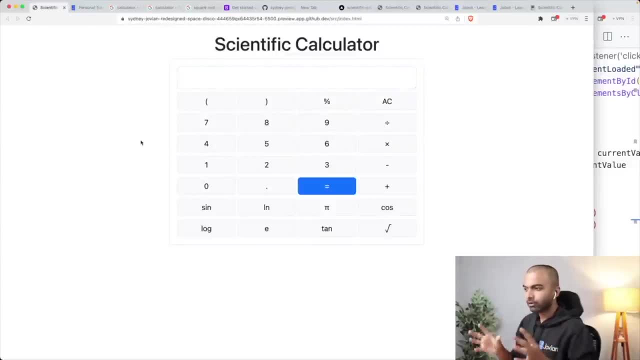 It's that you don't have to build in a lot of the complex functionality. you should always focus on building the most simple parts first, And then you can always add in the responsive design, the animation, the multiple rows of data, the history, etc. 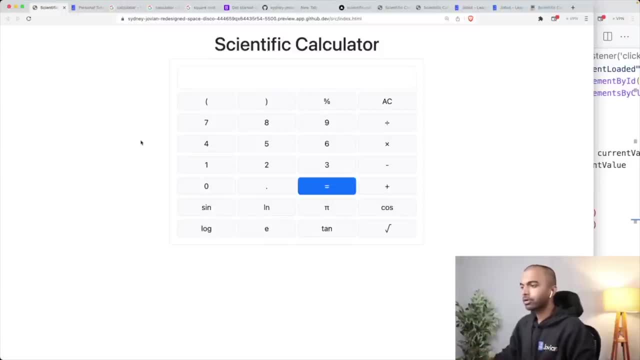 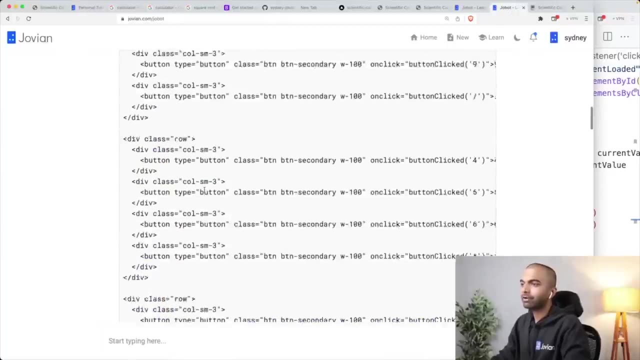 Those are all things that actually do require a lot of additional code, But the simple functionality is generally fairly straightforward to implement And in a lot of cases you can get a lot of help from from jobot, from chat, GPT, from whatever AI tools you're using. 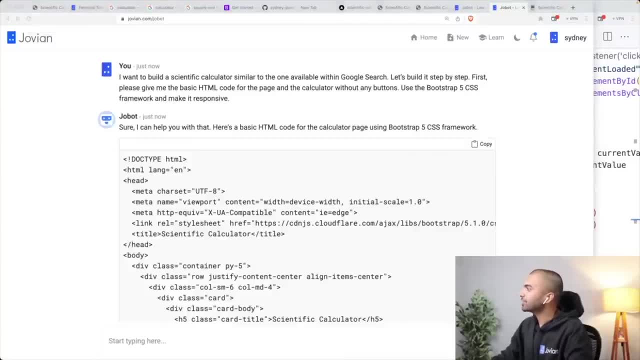 Okay, So let's see now if we have any questions at this point. Okay, well, I do not see Any questions. Can this be uploaded on YouTube? This is on YouTube. It's going to stay on YouTube, So you're fine. 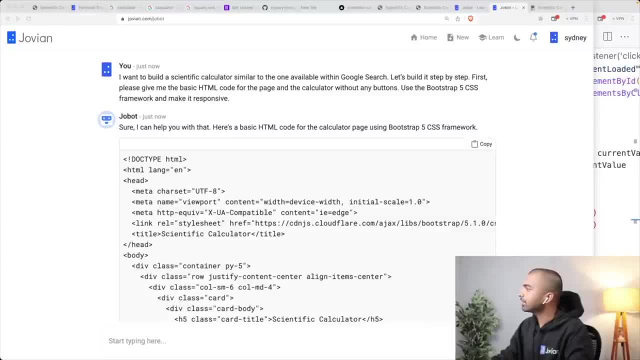 How to create a function for the, how to create a functionality of clicking on either effects or 123 and the buttons to ensemble changing entirely, Yep. So see, if you want to do something more complex than what we've done here, ideally what you 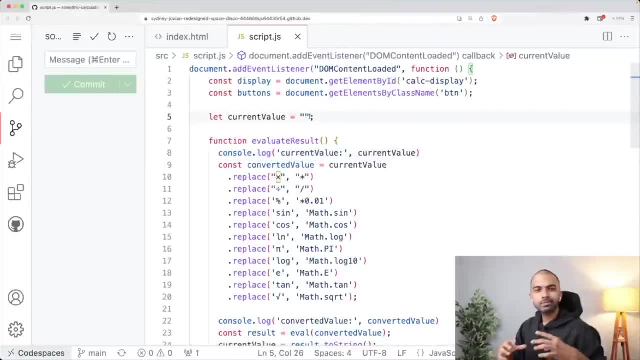 should be doing is two things. One, you shouldn't just be storing the current value in a string. what you should be doing is maybe having an. you should have an array of tokens. Okay, You should have an array of tokens, or array of hosting a value of button clicks. 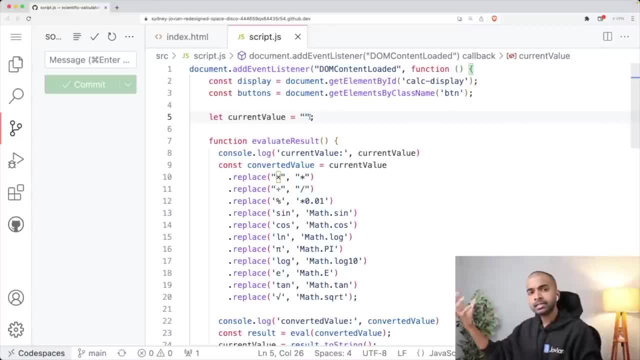 And that array could be converted into some value that is actually displayed in the input, So that when we click the equal to button you don't have to evaluate a particular string, But instead you can look at element by element. look, you can look at the array and you can. 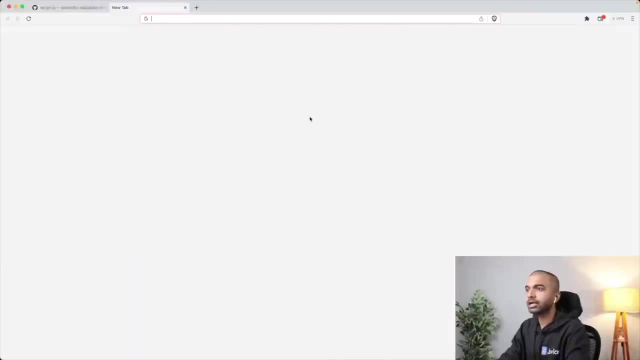 then use some JavaScript code to evaluate an arithmetic expression, right? So yeah, you could, for example: let's just try this and see what happens. Okay, Just try this. Okay, Jovencom, slash your word. you could, for example, ask your bot write a JavaScript. 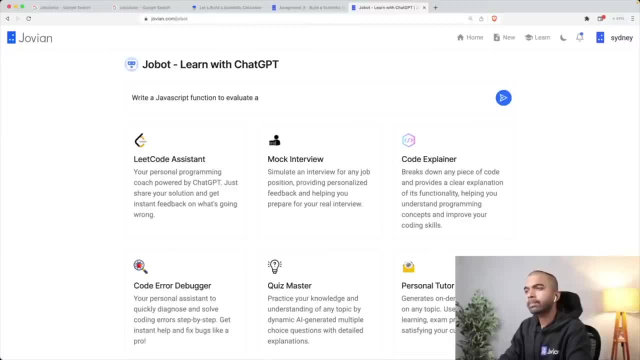 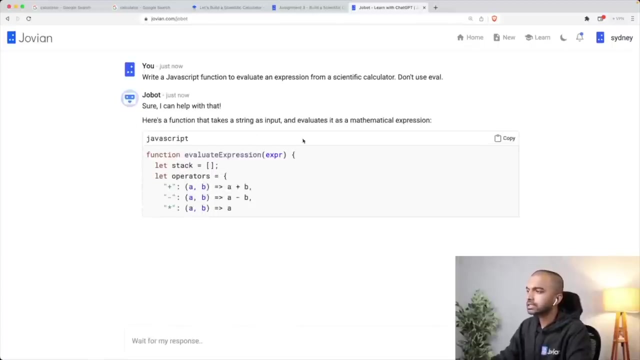 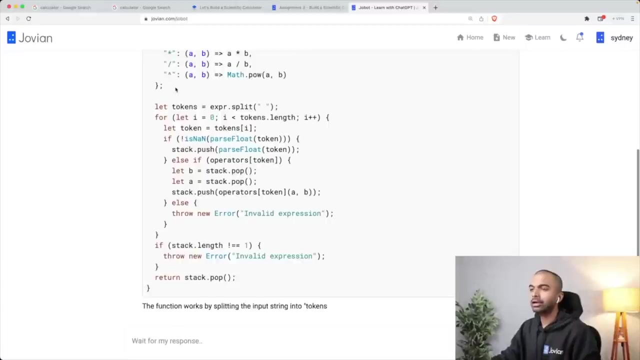 function to evaluate an expression from a scientific calculator. Don't use eval. Okay, Let's see. So this takes an input and it has this whole set of operators and you can add more operators as well. So you can see here that it has created a bunch of like basic code for you. 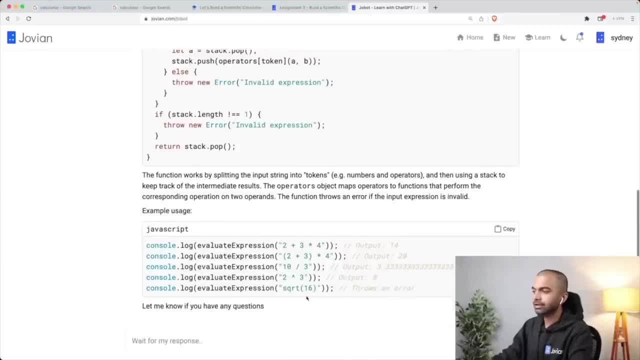 And now it's going to do some of this business And you can see here that it can work with all of these interesting operators. clearly, It could also potentially okay, square root is not yet supported, But let's say, add support for sign log, cos, etc. is going to then update that. 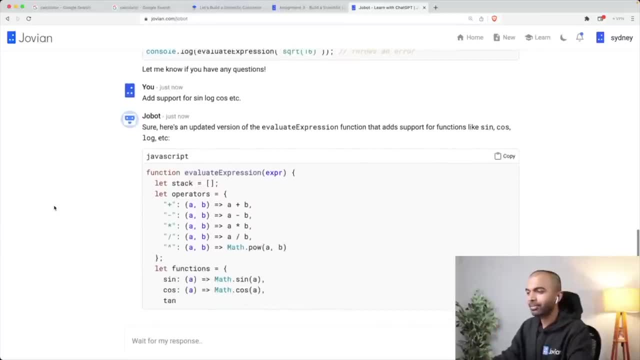 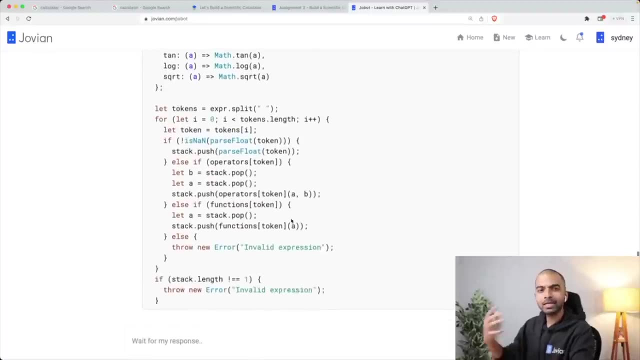 Let's see, Maybe we can actually use it in our code. Okay, I don't know, but possibly, yeah. So it's basically what it's doing. is it maintaining a stack? it is putting tokens into the stack, getting tokens out of the stack. 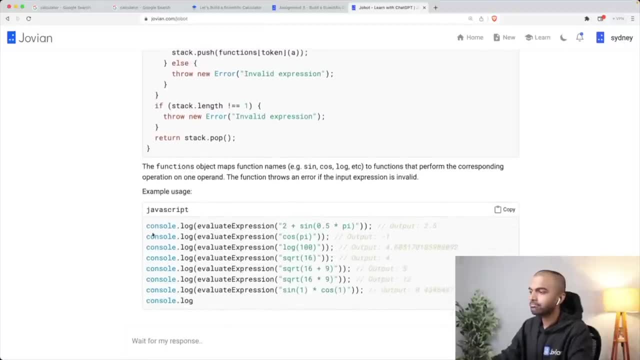 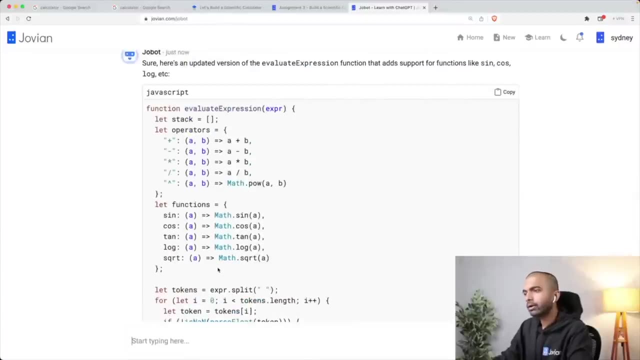 And it is also testing whether the expression is invalid. And, yeah, all of this should work. If all of this works, then potentially let's see if, okay, the maybe the expression may not contain any spaces, So we may have to fix that. 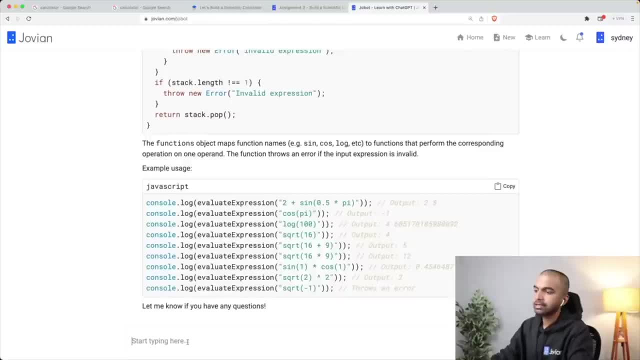 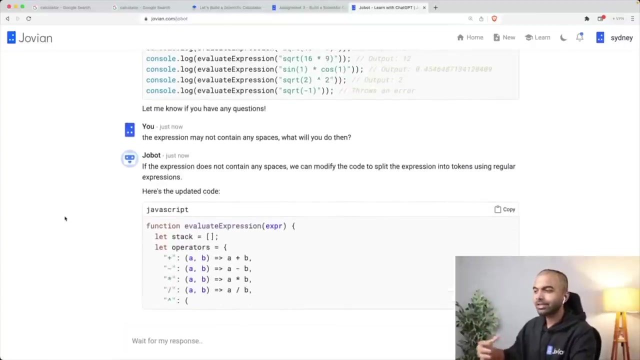 It says: let tokens equal, Let's say, like exprsplit space, the expression may not contain any spaces. what will you do then? Yeah, so it's going to write more complex logic and you can keep working with it and try to figure it out. 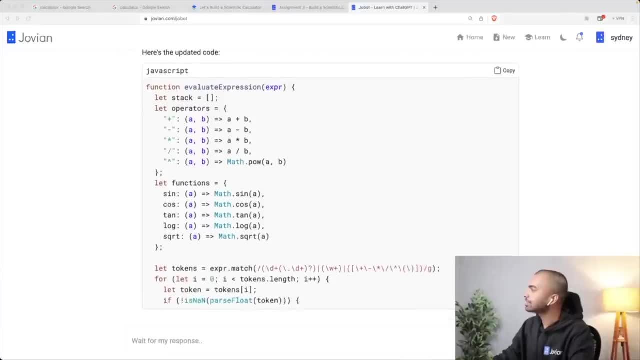 So I encourage you to try that out with chat GPT. Okay, instead of eval, you want to create a different function? Is there a battle ray? Yeah, So one thing you could do is you could actually attach on click handlers on specific buttons. 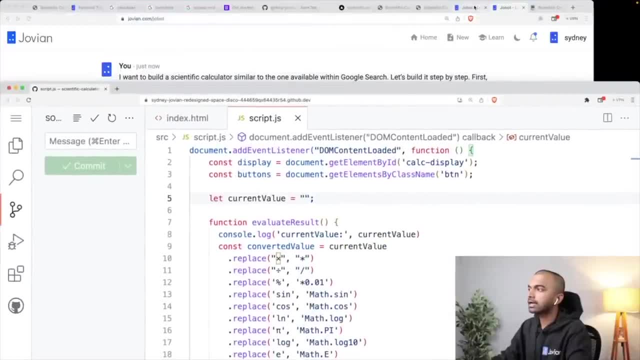 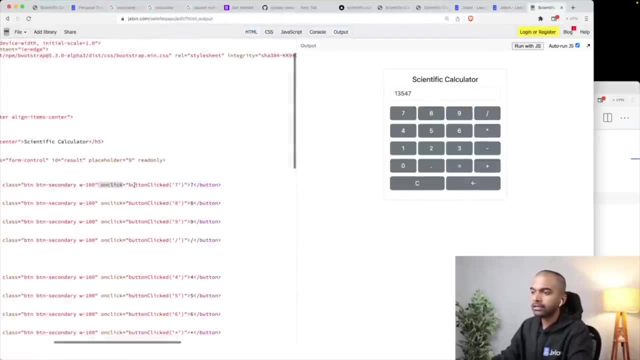 Okay, So you could actually attach on click handlers on specific buttons. Okay, So you can create functions directly from HTML. So I want to show you right here this is what cha, GPT or job, or tried to do. you can say on click and then you can provide the name of a JavaScript function that is defined. 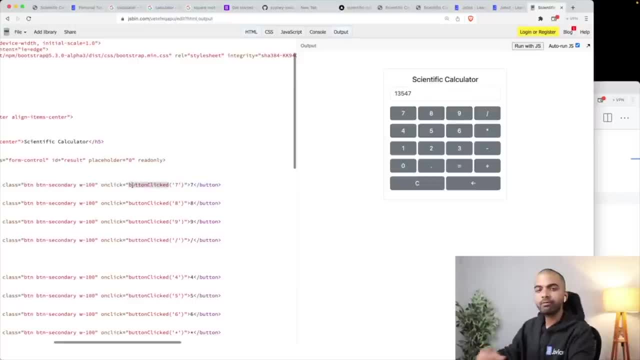 in the script file And you can call it with some value right, So you can have a function called button clicked and button clicked can be get called with this particular value when this button gets clicked. So that's one other way to do it. 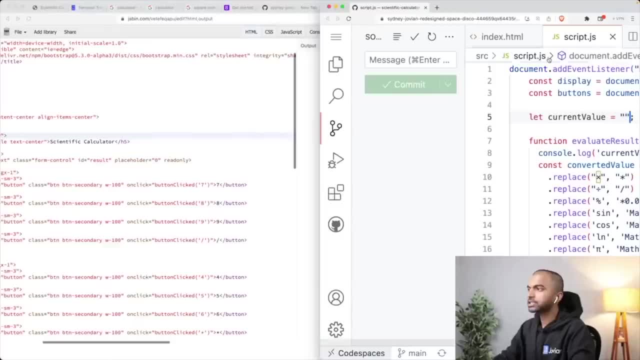 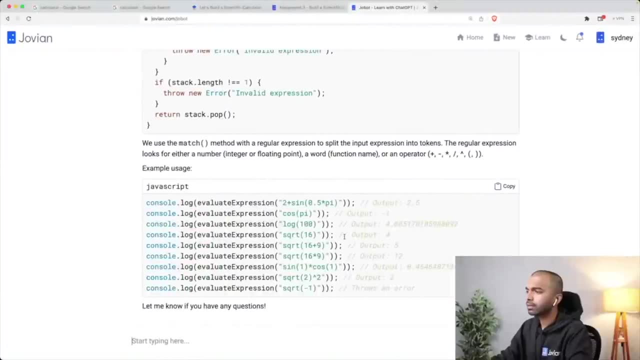 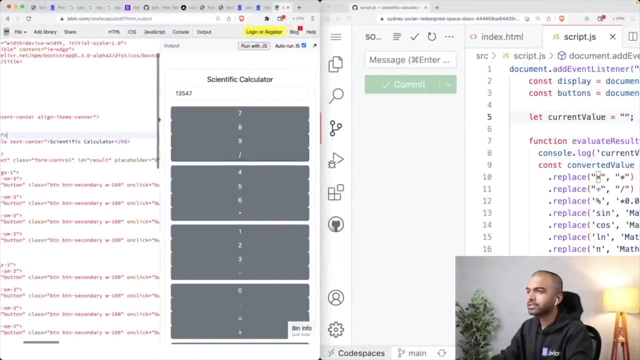 I am not going to go into a lot of detail with that right now, But just know that you can also specify on click handlers- handlers- within the HTML itself. So I hope that answers your question. Yeah, looks like this is actually working not too badly. Let's just try it out. I'm not sure if this is actually. 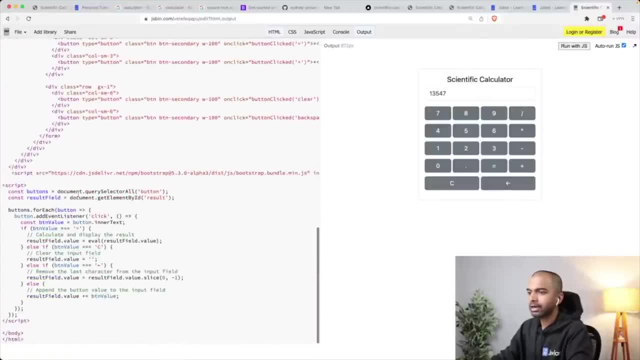 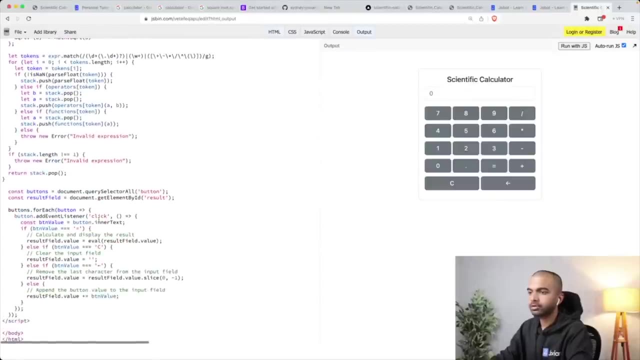 going to work. But let's see, let's put that in here. So let's get our evaluate expression And instead of eval let's just do evaluate expression over here. Evaluate expression. I should be taking a close look at this code, But what the hell? let's see seven times. 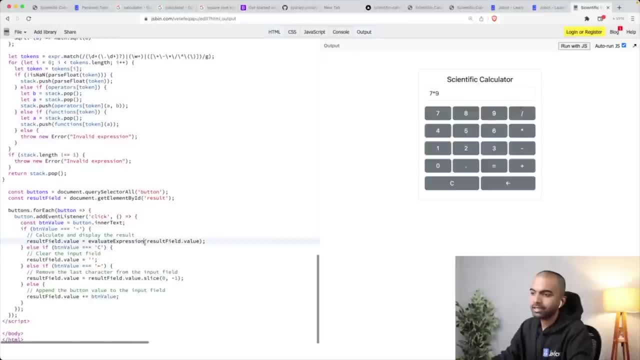 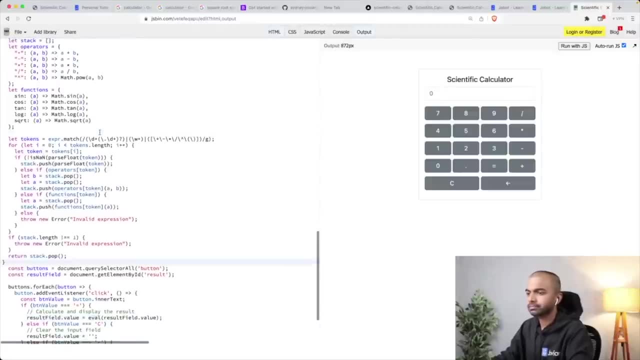 nine equals No. there's definitely some error here. I guess there's. it's not that straightforward, because it's like doing some regular expression: match Yeah. But now seven times eight works fine, Yeah. So you might need to just test this a little more carefully than what we. 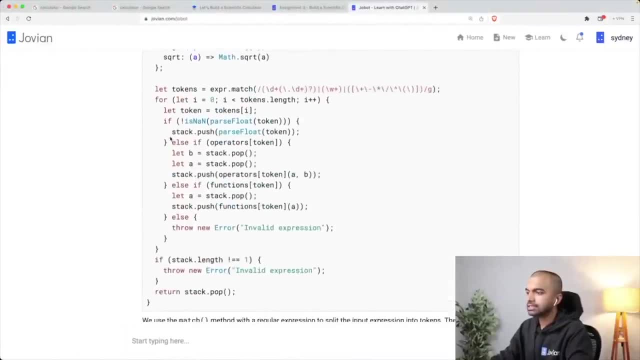 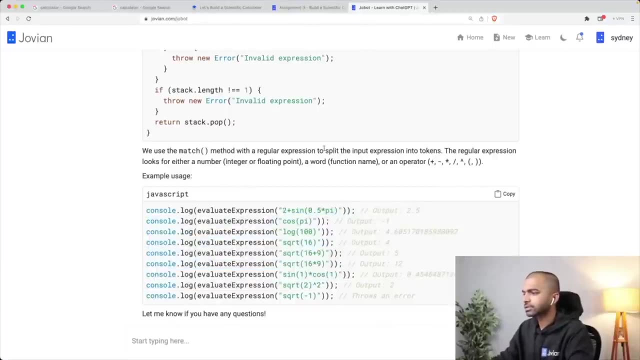 have done here, You can. one way to take test this would be maybe to put it into a JavaScript console and then test it out. But this looks, this looks good. I don't have a problem with this. With the modification, it should probably. 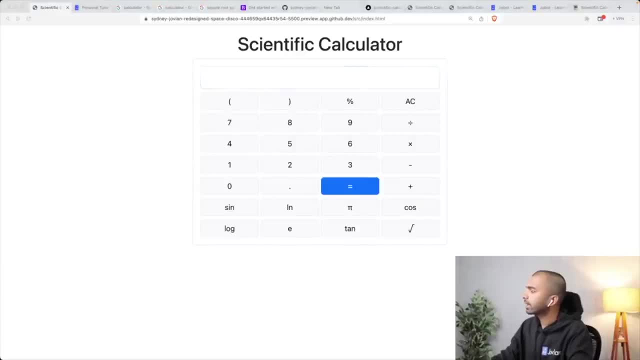 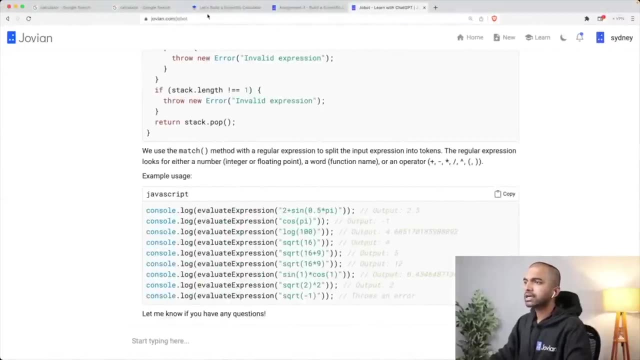 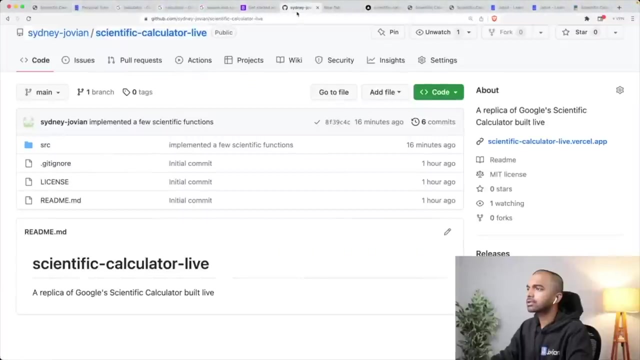 work out just fine. Okay, All right, I think that's everything that we were covering today, So let's just go back and check where we started. So we wanted to build a scientific calculator, And the way we did this is: let's grab those links and put them in here as well, so that 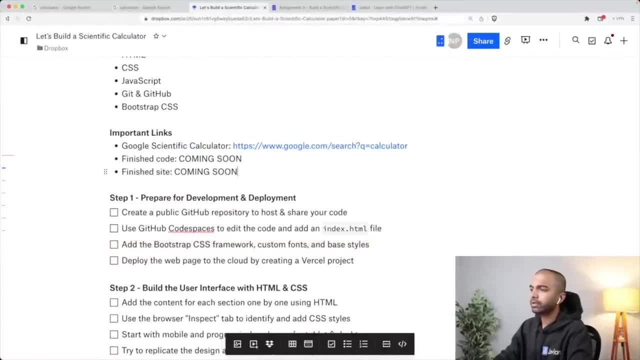 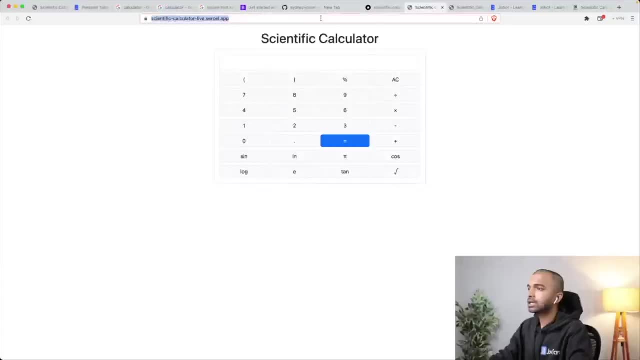 you can actually see these. So here is the finished code. I'm just gonna add it right here in this doc. It's also going to be in the description. Here is the actual scientific calculator that we've built out, the finished site. That's right here. 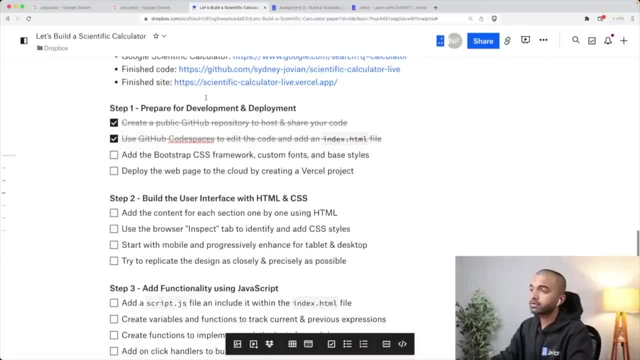 So we created a public GitHub repository, we use GitHub code spaces for development, we added the bootstrap CSS framework And, of course, we also later figured out how to deploy this webpage to the cloud by creating our self project, And you can then connected. 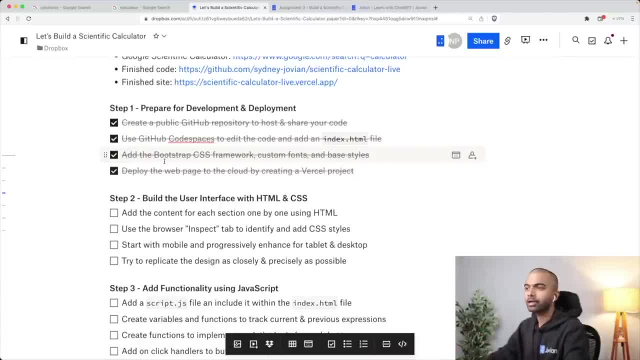 to your own domain as well. So let's go ahead and do that, And that's it. So we just created a public GitHub repository, So we use GitHub code spaces for development. we added the bootstrap, something like scientificcalculatorai or something. 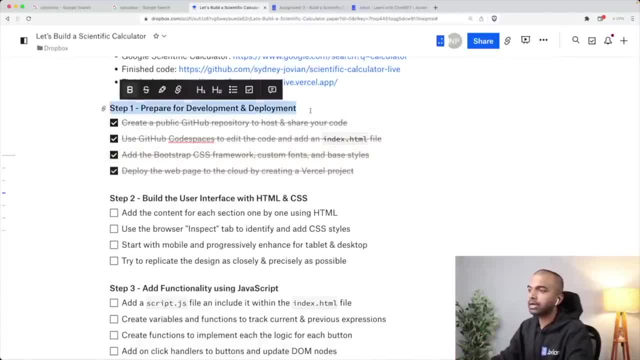 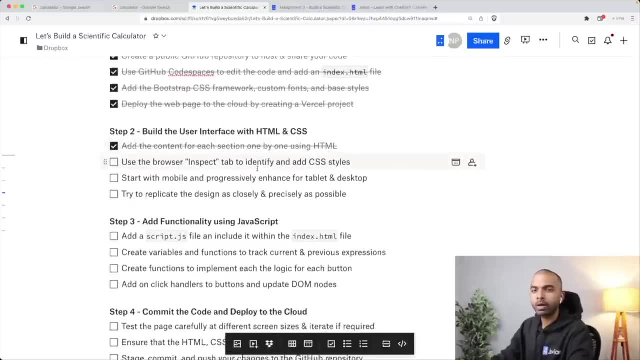 and it should work fine too. So that was the first step: prepare for development and deployment. The second step was to build the user interface with HTML and CSS, So we added the content for each section one by one using HTML. This is what it ultimately looked like. 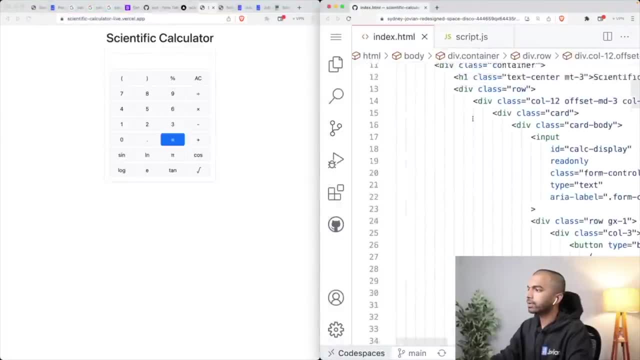 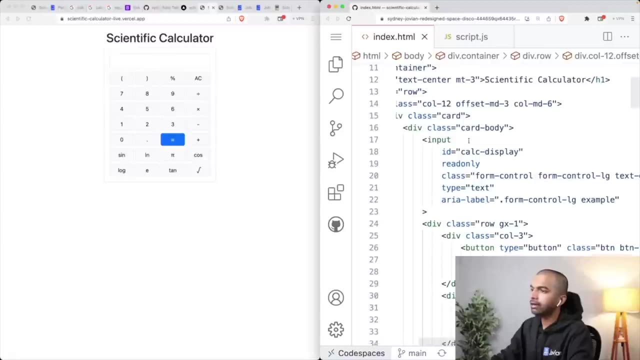 This was the HTML code. So we had a bunch of. we had like this row, we had maybe a column inside it, we had the title, we had a card, we had a body inside the card, we had an input. then we added the buttons row by row. 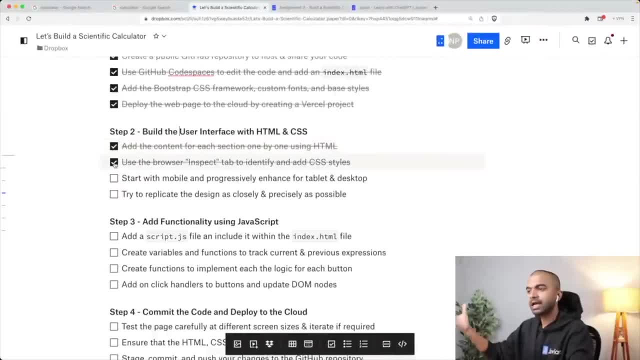 So we could also have used the browser's inspect tab on Google to inspect it, but we didn't need to do that. We didn't really get into a lot of progressive enhancement for tablet and desktop, but we did make it a mobile friendly or mobile first design. 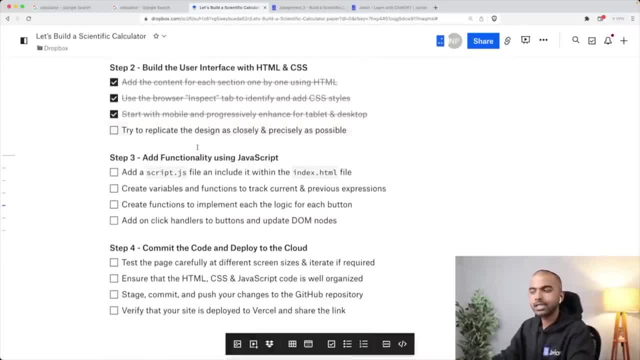 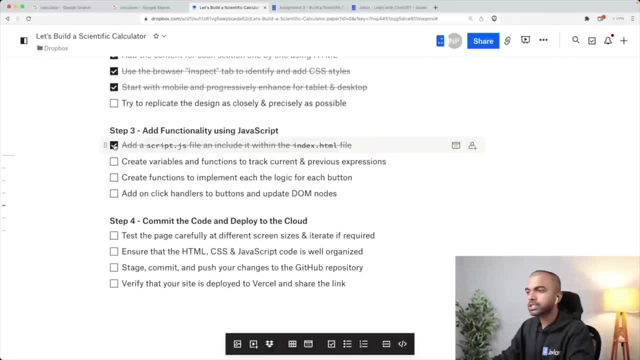 And we've not tried to design replicate the design very closely, but we did our best effort given the time we had. Then we did add a script file later in the process, but we started out simply with a simple script tag. The file was added later. 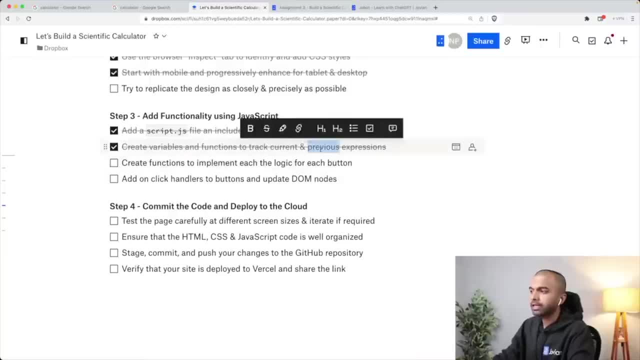 Variables and functions to track the current. we were just tracking the current expression. We didn't really track the previous expression. We added functions to implement the logic for each button. Well, it turns out we could just use eval and we did not actually have to implement the logic. 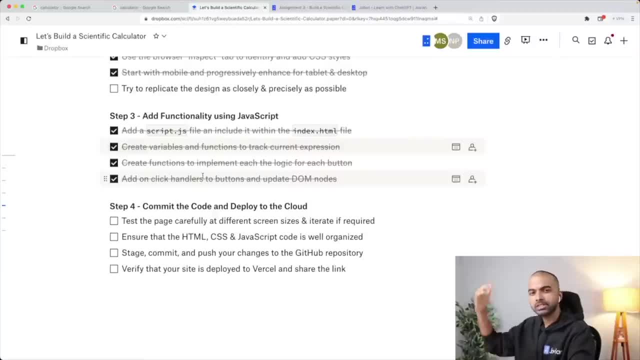 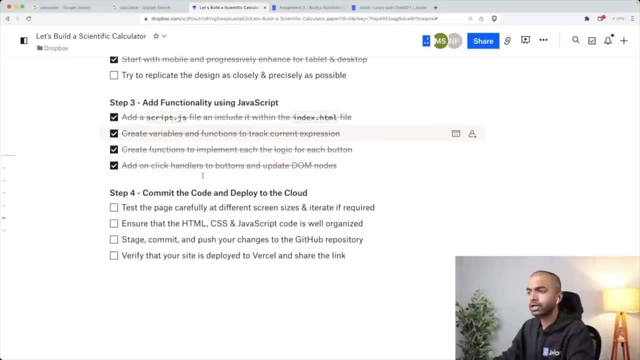 separately for each button And then on click handlers- those we just added it in a loop. So we took a bunch of shortcuts here, which is fine for something like this, Where there is no sensitive information for us to worry about. we just used eval. 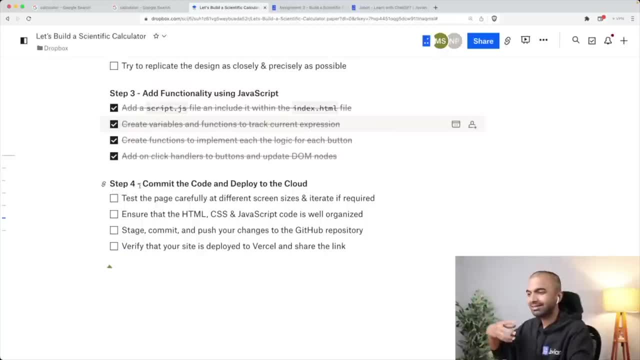 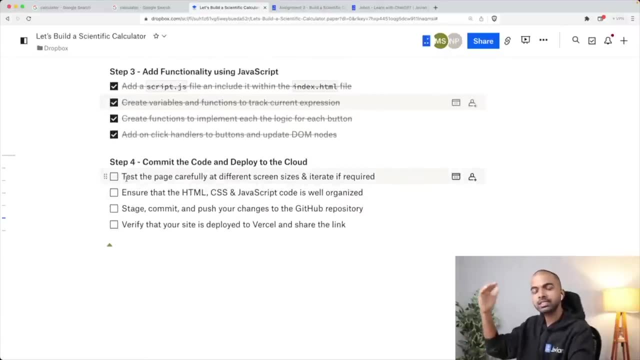 But otherwise you might want to use an evaluate expression kind of a formula or an evaluate expression function again could be generated with help from Jobar. You could also give it some example inputs, saying these are some example inputs you have to handle And giving the 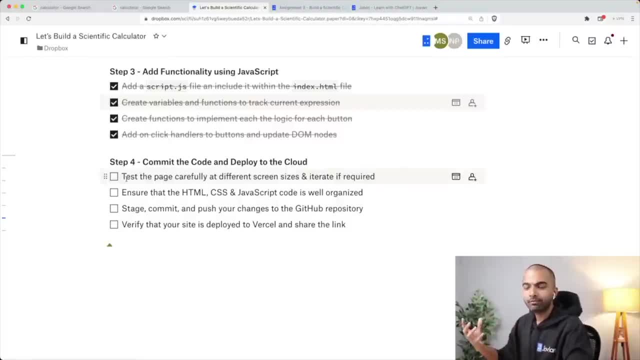 keeping those example inputs in mind, it's going to then generate a function. So remember that it's not always going to be able to read your mind and know exactly what you need. So you need to give it some input, need to give it some examples And in a lot of cases you can also give it if it does not give. 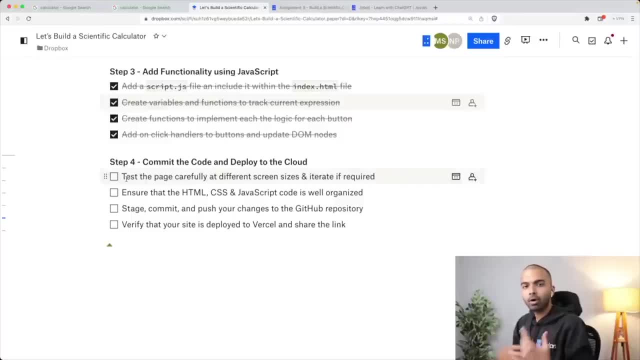 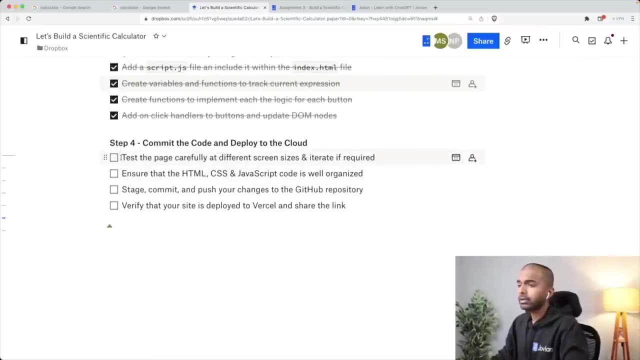 you exactly what you want. you can then ask it another question, follow up with it and it can give you the right answer. And you can also just copy paste your error and it'll fix things for you. Okay, And of course, you should very carefully look at all the code that is generated by AI. 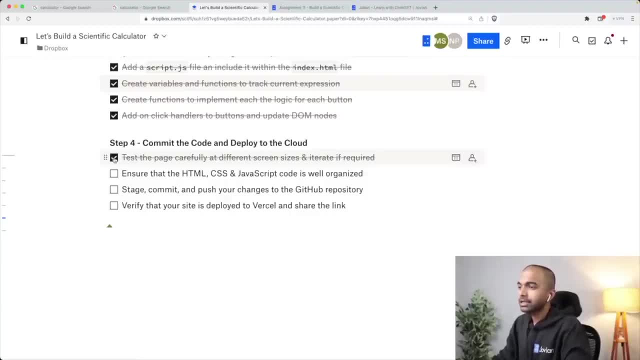 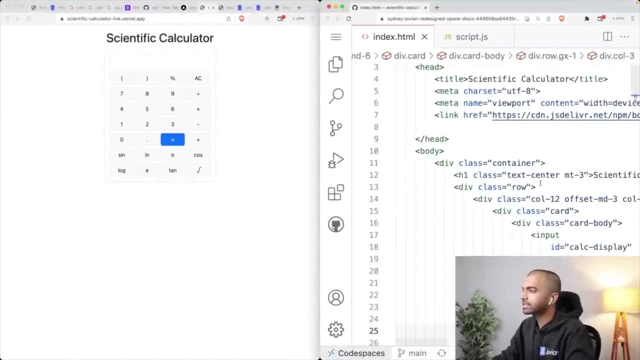 definitely don't just copy paste the code into your projects. Okay, test the page carefully at different screen sizes. Ensure that HTML CSS JavaScript is well organized. Yeah, it looks fairly well organized to me. I could add a few comments here and there. Maybe I could add a few. 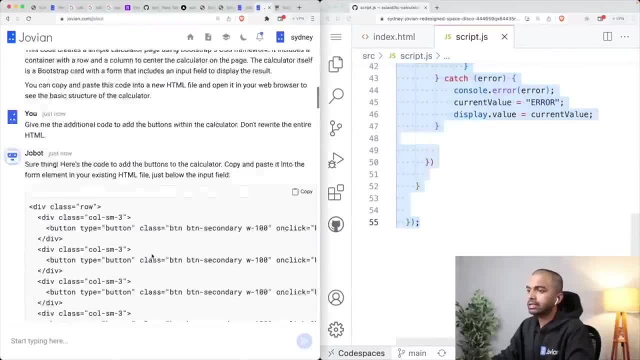 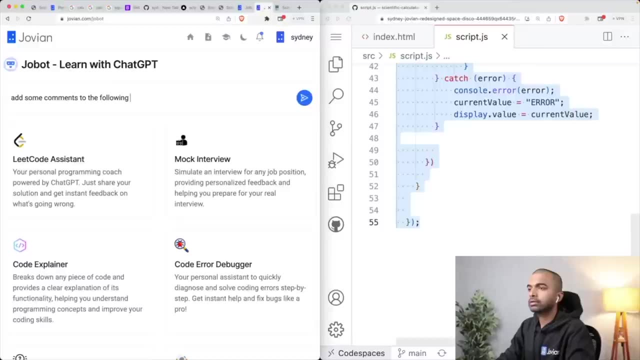 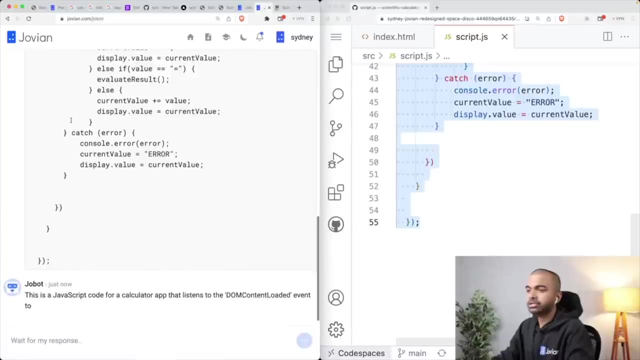 comments here. So I could always just go in here And I could say to job art, add some comments to the following JavaScript code, And it can add a bunch of comments for me. Yeah, it is not explaining the code, but I want to. 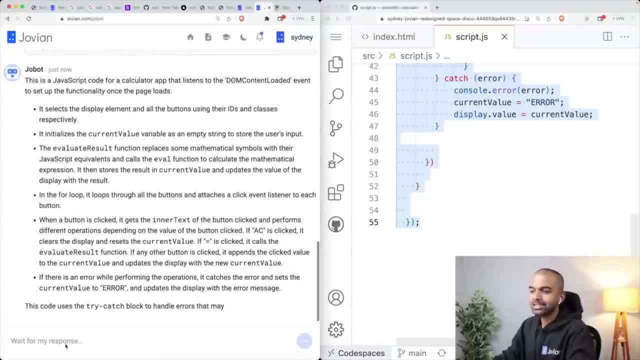 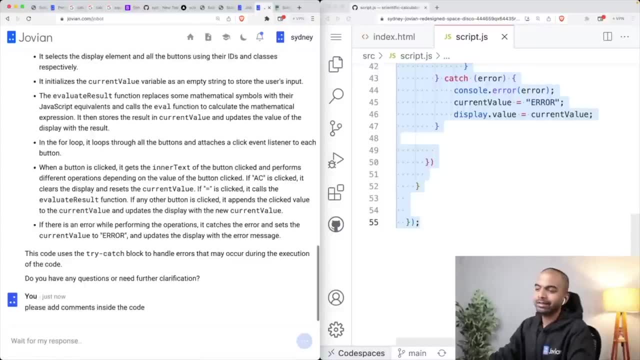 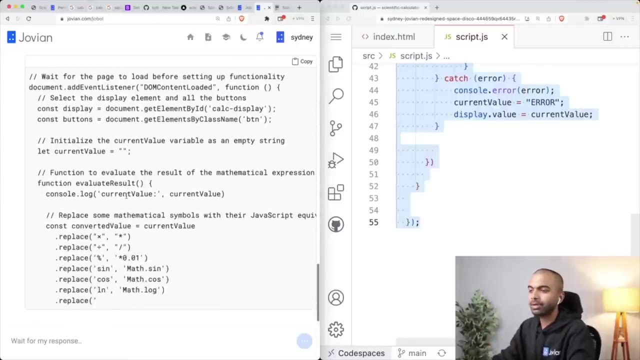 add. I want to add some comments inside the code And I can always tell it that, Yeah, please add comments inside the code. Okay, so it may not understand. it may not exactly understand what you want it to do, But just talk to it, just don't give up immediately. And now it is rewriting the. 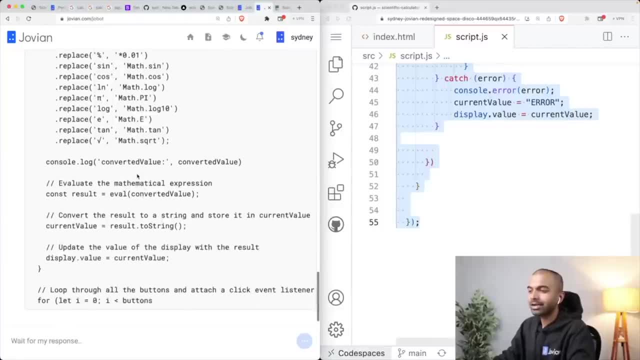 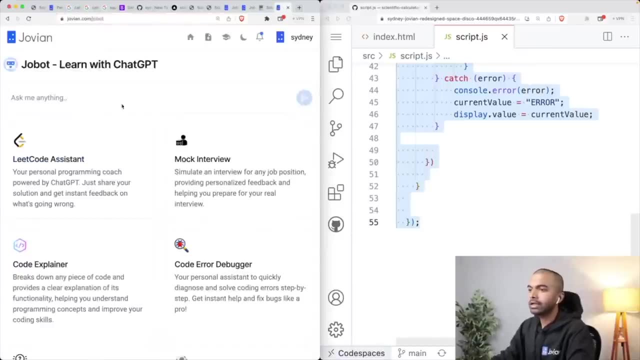 code for us with a bunch of comments. How nice is that? All right, And one thing you can also do is you can just use your bot to get explanations on code. So you can always just go on joviancom And simply go on code explainer and paste whatever piece of code you have. 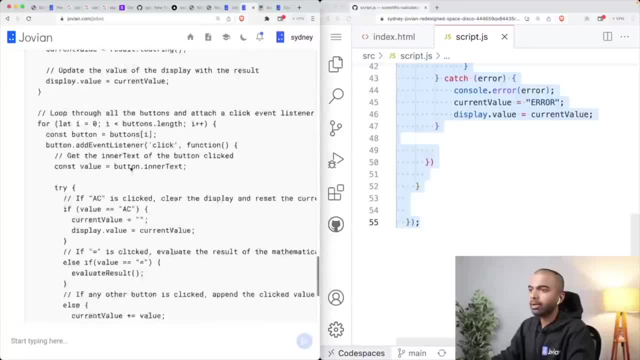 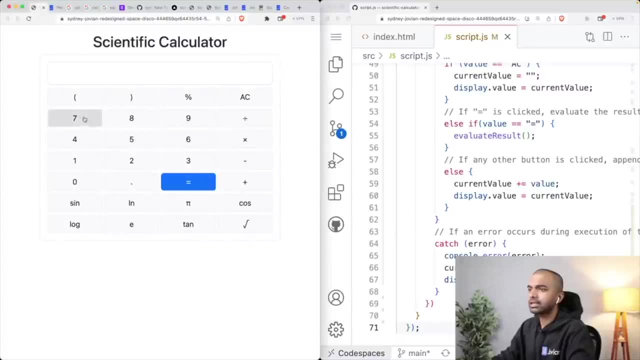 enter the programming language and it's going to explain that code to you. But let me just for now, let me just take this code, put that in here and see if it still works. I think it should. I don't see any reason why it shouldn't. 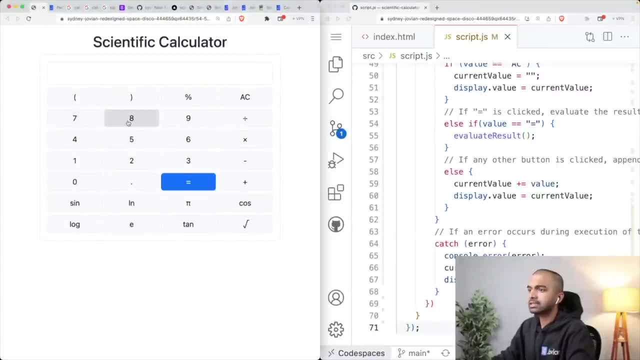 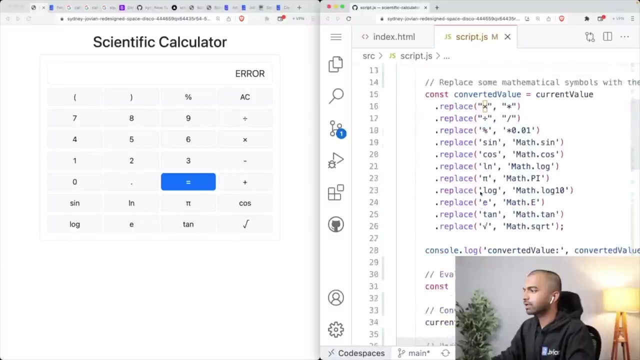 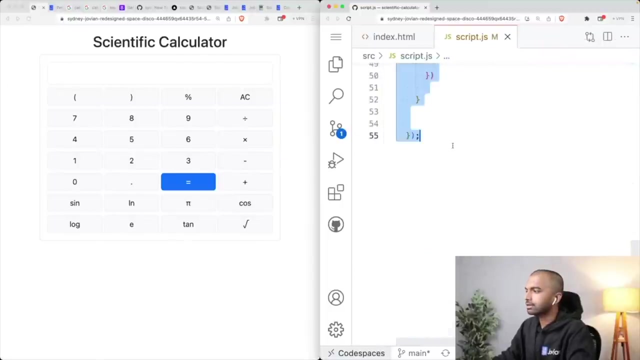 generally doesn't mess this up too much. Let's see: 888 minus three equals 85.. Yep, Ellen, let's do AC Ellen. Eight, it should be about. okay, Ellen seems to have failed. Yeah, for I'll investigate that later. But yeah, you can definitely use it to document your code. 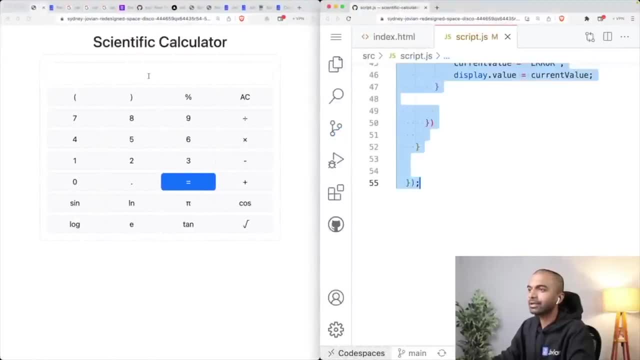 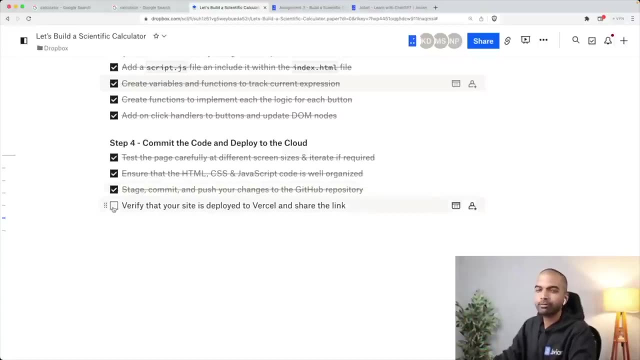 as well. Just verify that it has not modified any of your existing code. Okay, so that we did. then we staged commit and push star changes all in a few clicks on VS code. didn't have to write any git commands. And then we verified that our site is deployed to our cell. we tested. 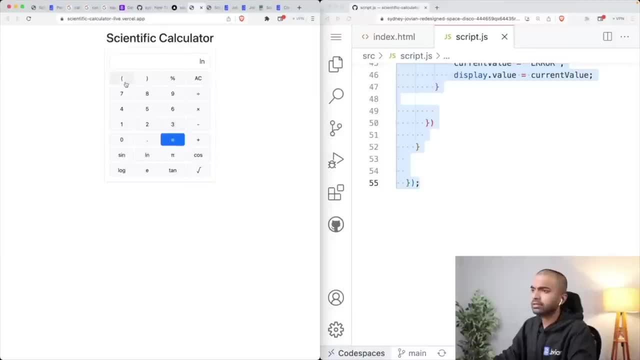 it out And it's working fine. Again, maybe there might be something I might need to fix. Yeah, there's something wrong with my Ellen function Cannot read properties of undefined log 10.. Yeah, I guess it's probably math log 10.. 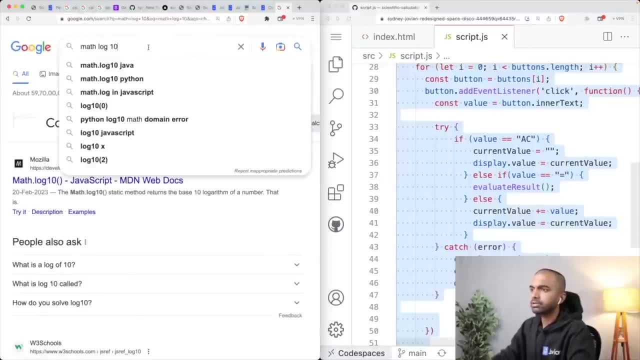 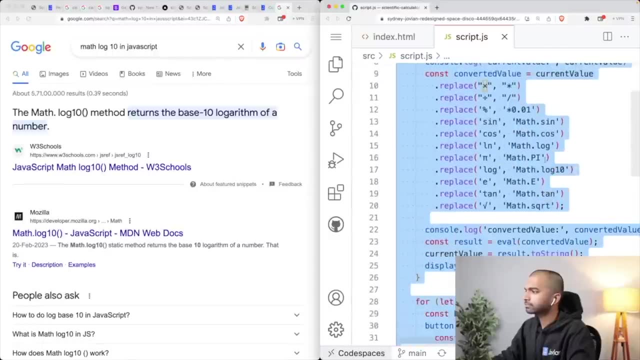 There's something wrong with that In JavaScript Math dot log 10.. Hmm, Okay, I don't know what's what's going on here, but we'll fix it. We'll find it and we'll fix it, No problem. 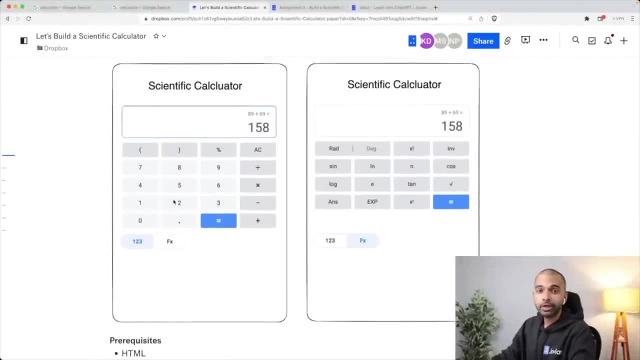 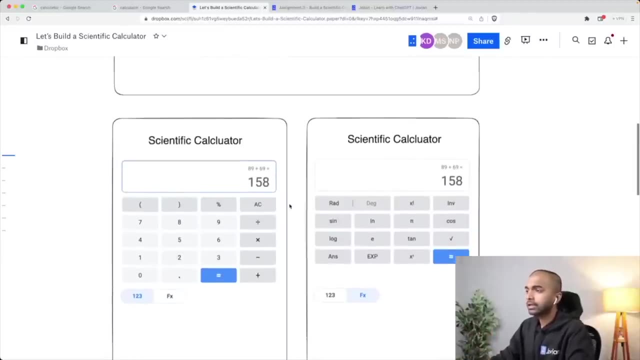 So with that we've reached the end of this tutorial. I hope you enjoyed it. Do leave a like on the video And, of course, please do subscribe. We're going to do more of these tutorials And if you have any questions, please post a comment. We will try and reply to. 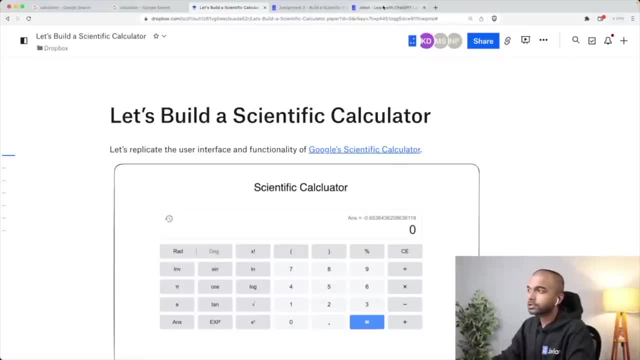 all the comments, specifically if you have technical doubts, Or you could also just go on jobincom, slash jobot, and ask your question And we'll see you in the next video. Bye. Thank you so much for watching. I'll see you in the next video. Bye. 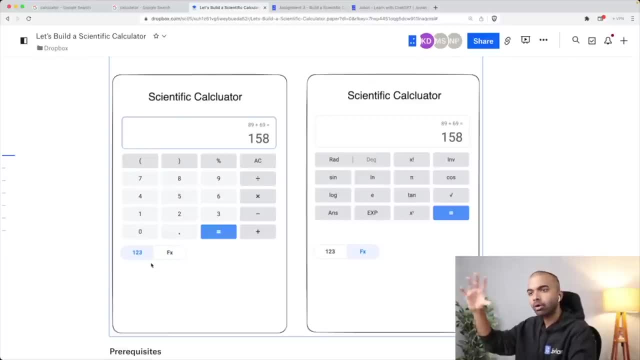 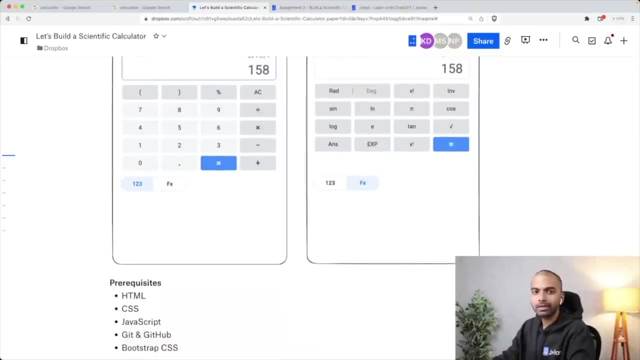 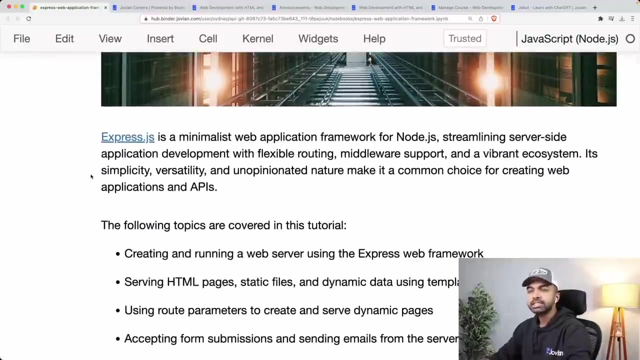 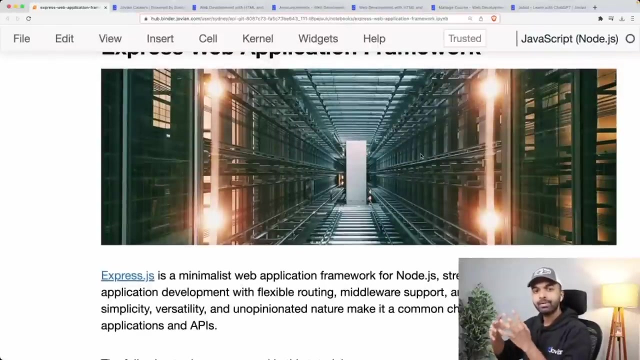 Thanks for joining and have a good day or good night. Take care, Don't make sense right now. Now, you might think that a server is a piece of software, And that is partly true. server is some is a piece of hardware, And you might think that a server is. 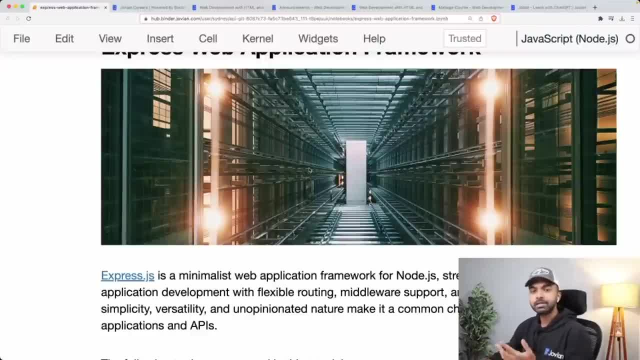 a piece of hardware, And that is partly true. These are racks of servers in a data center, But the server that we're going to talk about today is a piece of software that serves requests. Now here's what we're going to cover in today's tutorial. we'll talk about creating and running a. 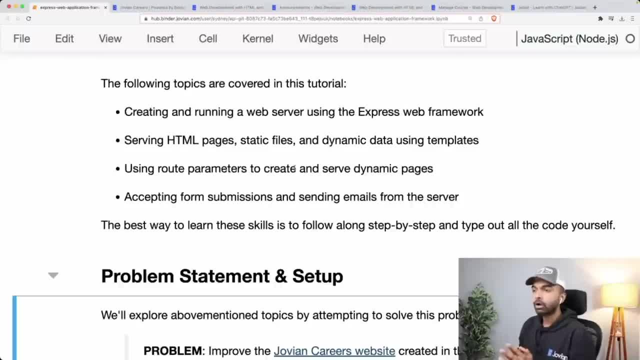 web server using the Express Web Framework. We will talk about serving HTML pages, static files and dynamic data Using templates. we will talk about using route parameters to create and serve dynamic pages. We will talk about accepting form submissions and sending emails from a server. So 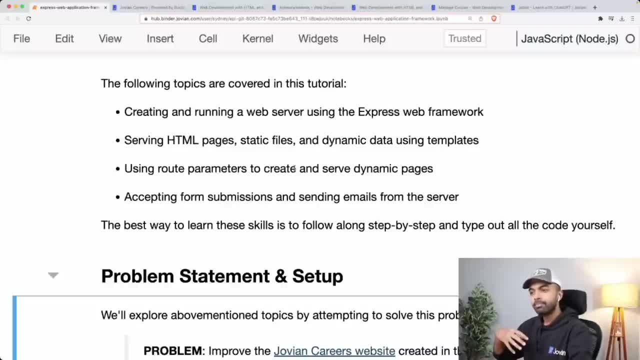 there's a lot of ground we're going to cover today And in some sense we are stepping into the full stack domain here. In some sense, we are covering the back end side of things now that we've learned basic web development. So let's move forward. Now we're going to talk about how we're 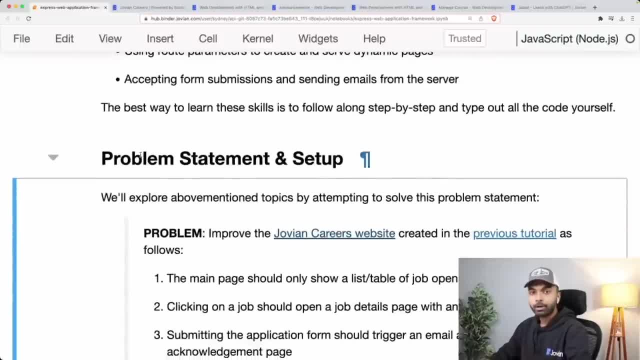 going to use the Express Web Framework, And we're going to talk about how we're going to use the Express Web Framework. Now, of course, the best way to learn these skills is to follow along step by step and type out all the code yourself, So make sure to do that to get a proper understanding. 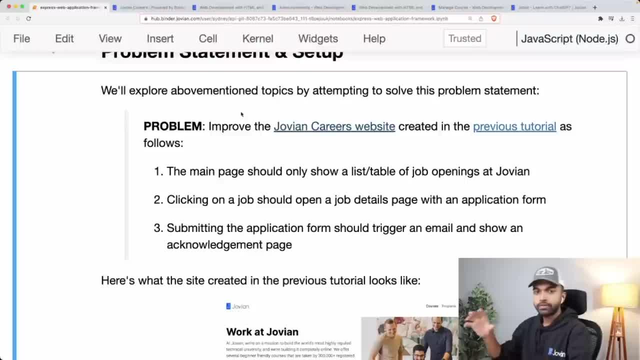 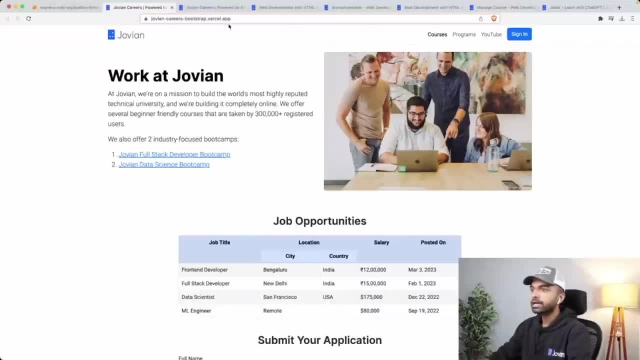 And we will explore these topics by attempting to solve this problem statement. So the last time we created a Jovian careers website powered by bootstrap- and this is what it looks like- It has a navigation bar. it has a bunch of links here in the navigation bar and a sign in button. 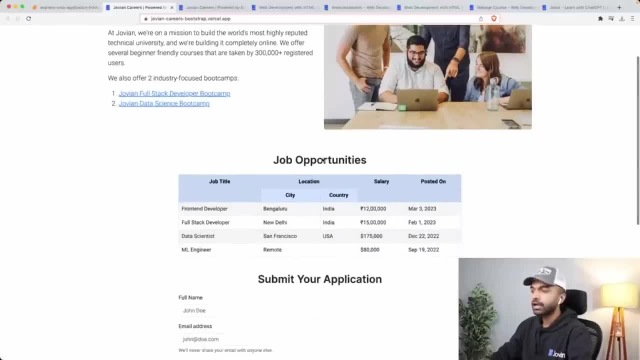 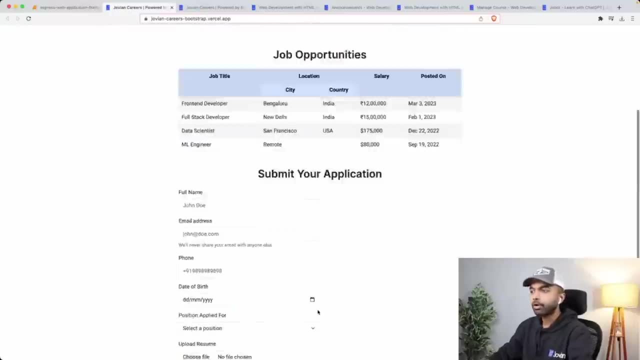 it has this work at Jovian section with some text and an image, And it has this job opportunities table, a list of job opportunities and a list of job opportunities. So let's get started. opportunities and an application form, And it has a footer here at the bottom. Okay, 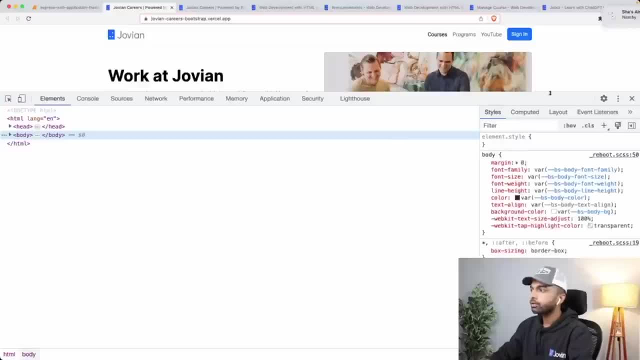 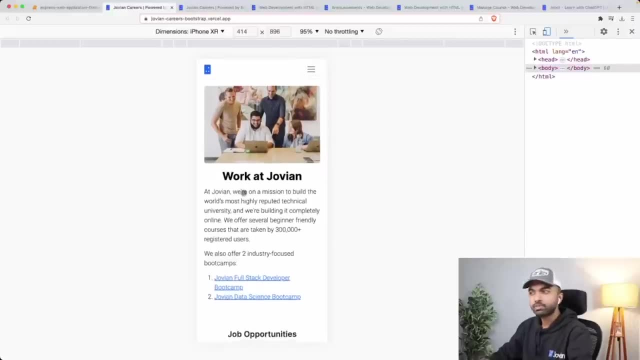 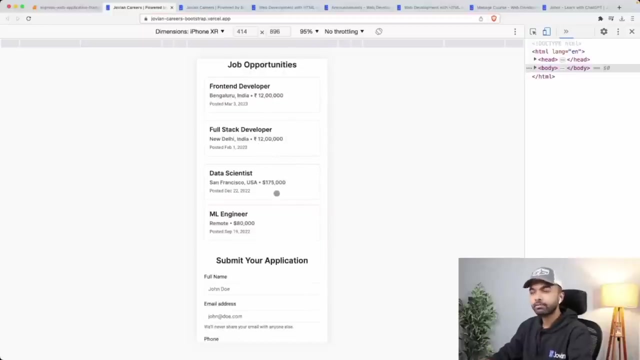 so we built all of this using bootstrap And you might also remember- you might also remember that we had made this responsive, So you can see here that there's an image here, at the top there is some text And on the mobile view, we have cards instead of instead. 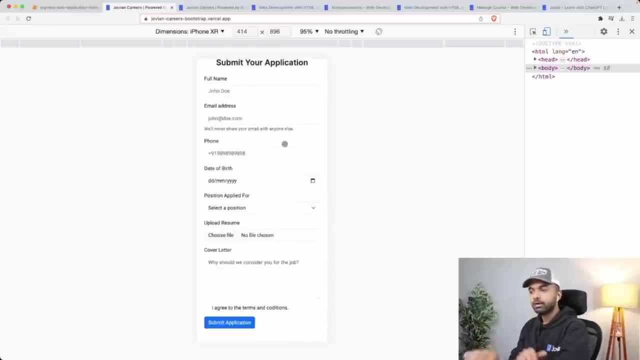 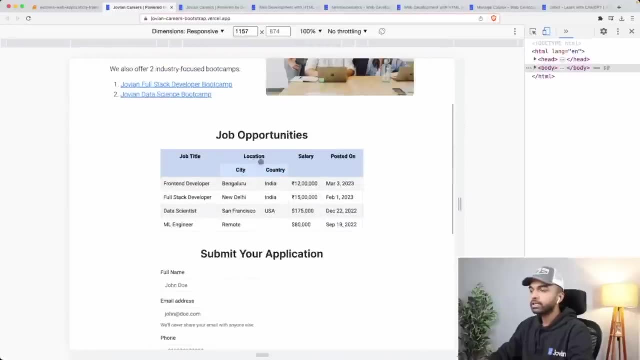 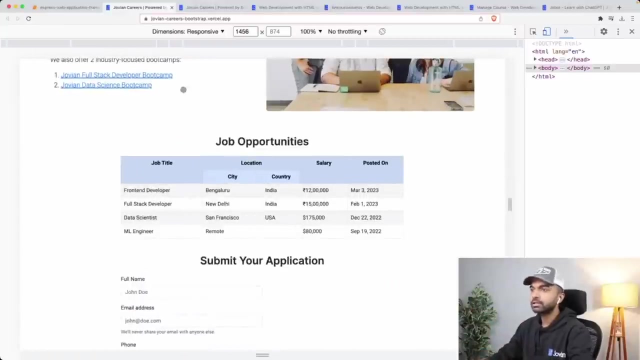 of a table And we have the same application form, except that it is now adjusted to show up properly on mobile And it scales properly as we grow from mobile to tablet, where we switch into the job opportunities table from the job opportunities card list and then we also take up more space on the screen. 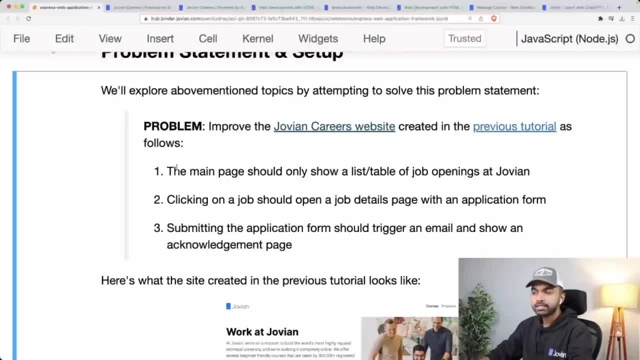 Okay, now we are going to do a couple of things this time. the first thing is that we should we want to make the main page only show a list or a table of job openings. we do not want to have the application form on the same page. It's probably a better idea if clicking on a particular 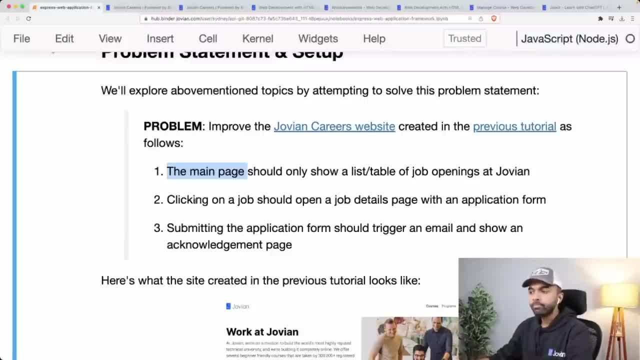 job role opens a job detail. So if you click on a job role, you can see that the job details are already there. We can also see that the job details are already there. So if you click on the job details page with an application form, and submitting that application form can then potentially trigger an. 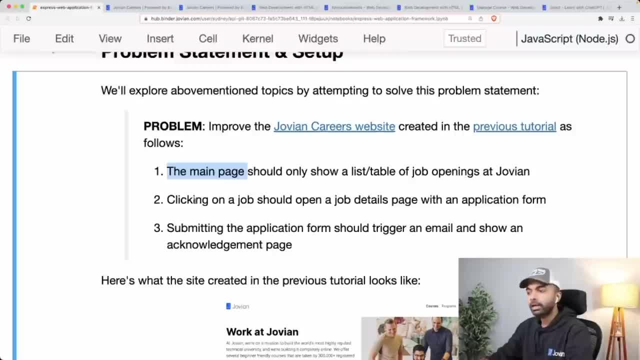 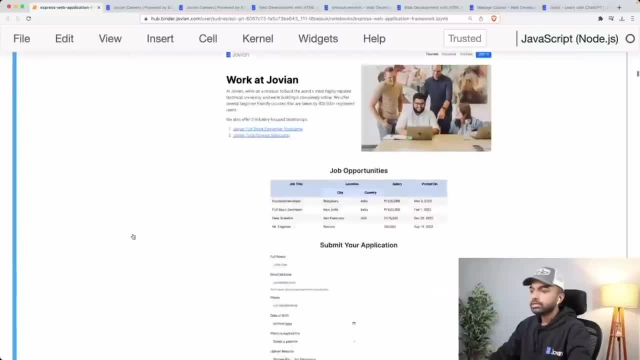 email to us and also show an acknowledgement for acknowledgement page to the user. So now we're going to build a server which is going to accept these form responses and send out an email. So let's get into it Now. of course, we assume here that you have knowledge of HTML and CSS. 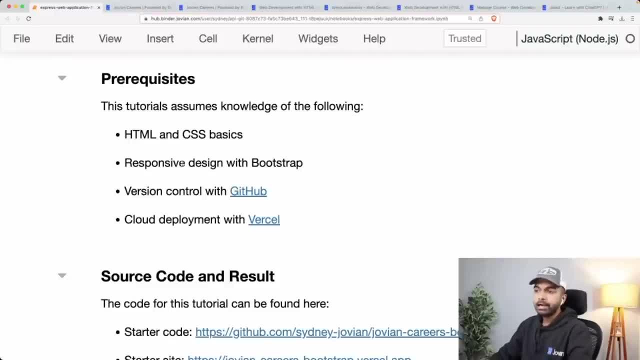 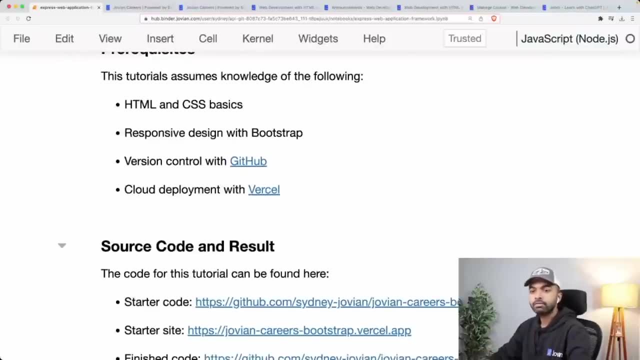 basics and responsive design with bootstrap, And you are familiar with version control with GitHub and cloud deployment with Vercel. Okay, So, let's get into it, So, let's get into it, So, let's get into it. If you haven't, please make sure to review the previous lessons before we move forward And you. 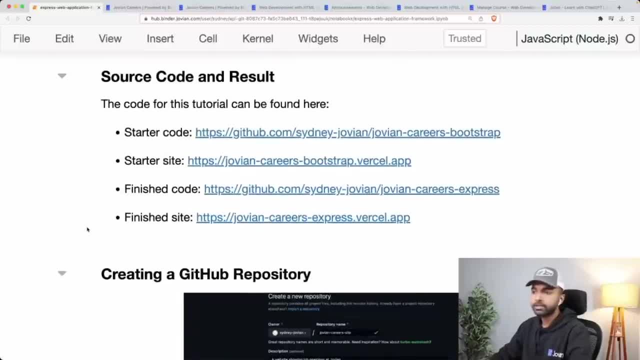 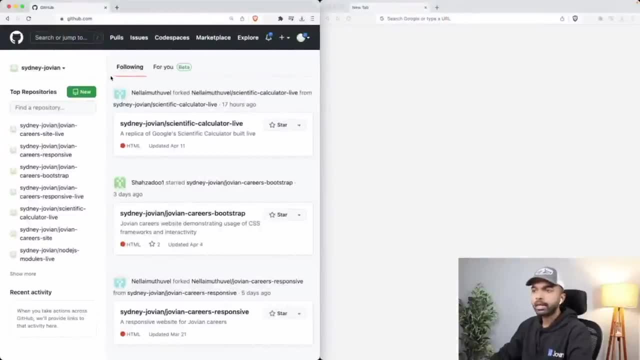 can find all the source code and the result for the starter site and the finished site over here in the notes. So we start by creating a GitHub repository. So I'm just going to go over to githubcom And if you're not signed in, make sure to sign in And I'm going to click new. 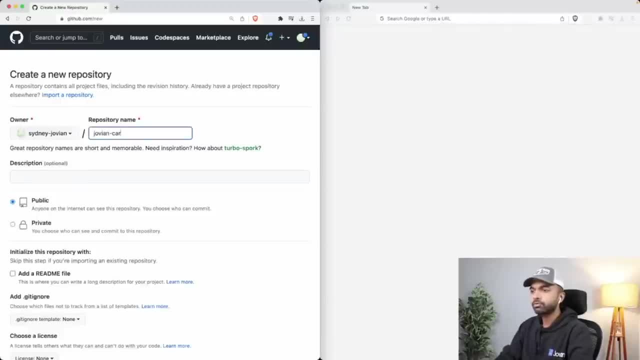 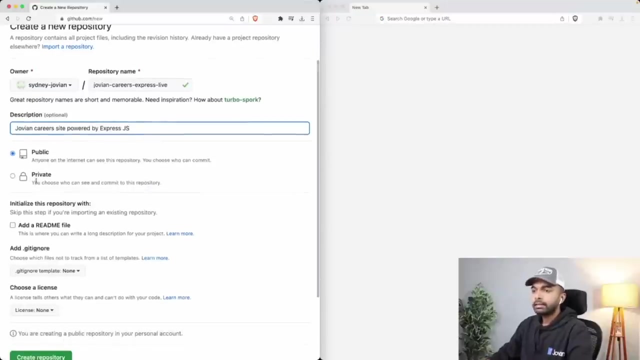 And I am going to create a repository, and let me just call this Jovian careers, Express life, because we're building this life And this is simply a Jovian career site, tall burden by ExpressJS. All right, and this is going to be a public. 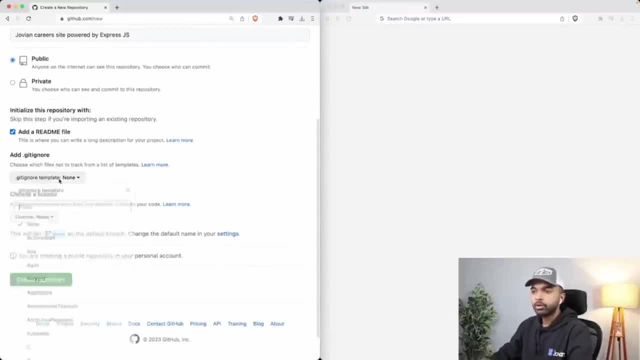 repository. I am going to initialize it with a readme file, I'm going to select the getting ignore template node js, because we're going to actually write some NodeJS code this time, And I'm going to give it the MIT license And let's create that repository. 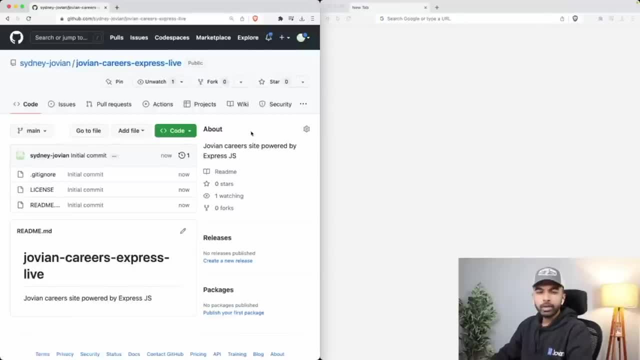 So, with that, repository is now created And now we need to. now we need a way to run this repository. Of course, you can download this repository onto your computer and run it, but we are going to run it using Codespaces and I just select the code option here and select Codespaces. 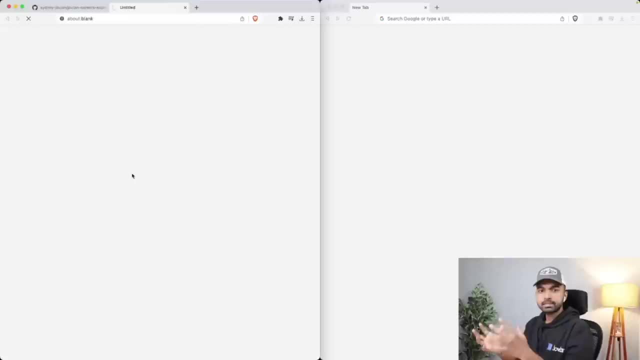 and click create Codespace on main, And what this does is GitHub sets up a machine for us on the cloud where it pulls the contents of this repository and opens up a Visual Studio Code interface for us to interact with the repository, which is to write code and run the code, test things, and then we can. 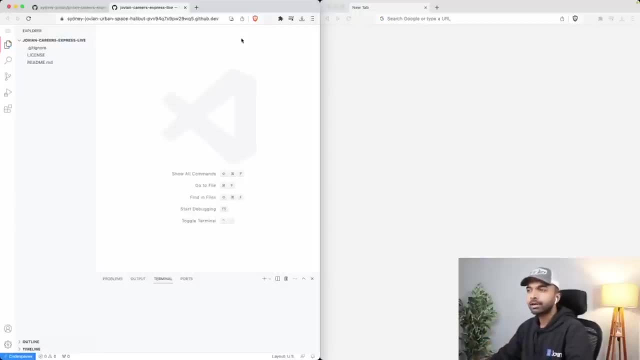 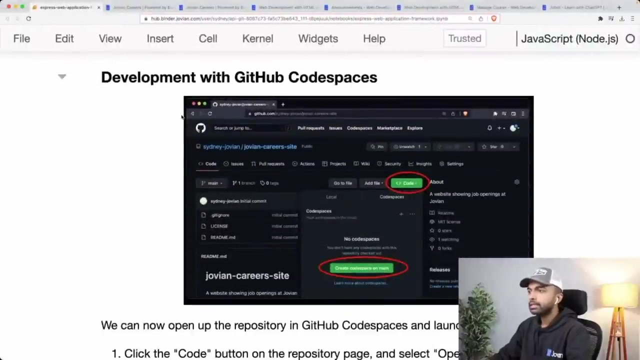 push these changes back to the GitHub repository. Okay, so that is a GitHub workflow that we have been following for the past few lessons. All right, let's give that a second to start properly. Now let us- so here's what you do- to start developing on GitHub Codespaces. 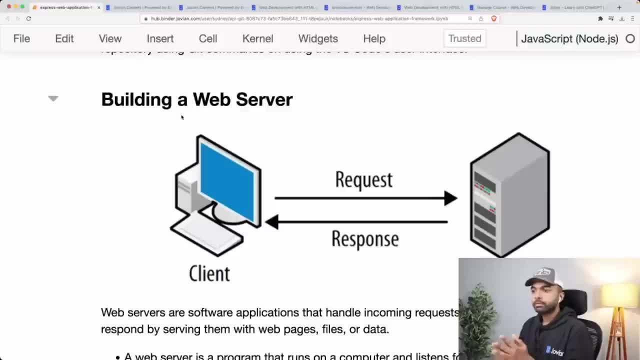 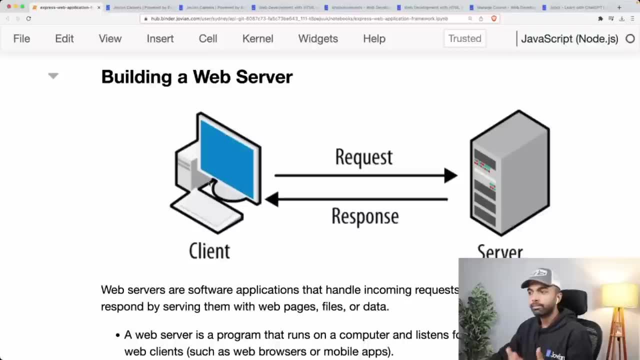 And now let us start building our web server. Now. web servers are software applications that handle information. So a web server is an incoming request from a client, and that client could be a web browser, or that client could be a mobile application, or that client could be a Discord bot, Slack. 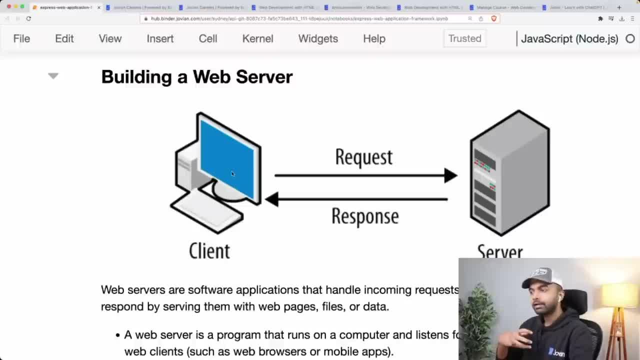 bot, anything, any form of a client, anything that requests or needs some information, makes a request to a web server and then the web server processes that request And for processing the request it may then contact a database. it may contact another. 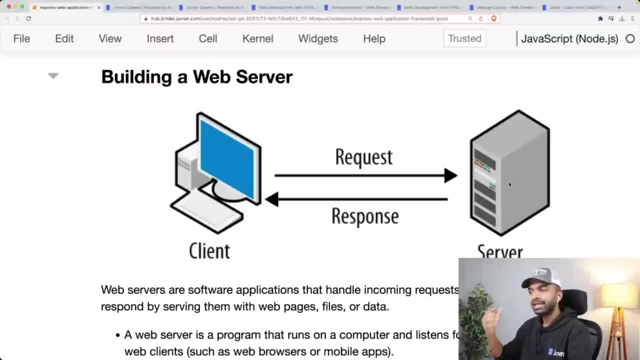 external service. it may do some data processing and then it returns that response back to the client. All right, So there is a request sent from a client, some processing happens from the server and the response is sent back to the client. 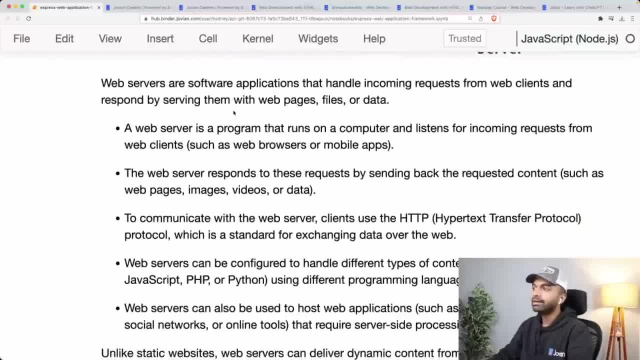 So that's basically what a web server is: software applications that handle incoming requests from web clients, And it runs on a computer. essentially So, a web server is running on some computer on the cloud and is handling incoming requests And it responds to these requests by sending back the requested content, and that could. 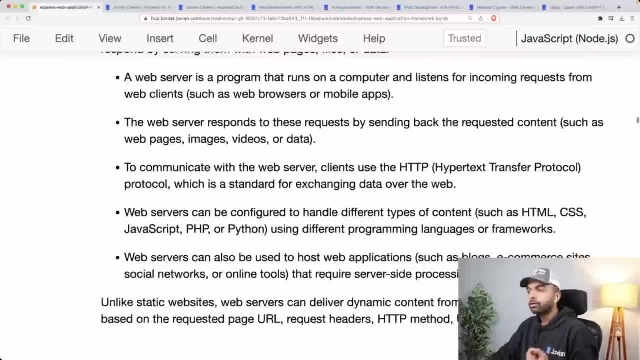 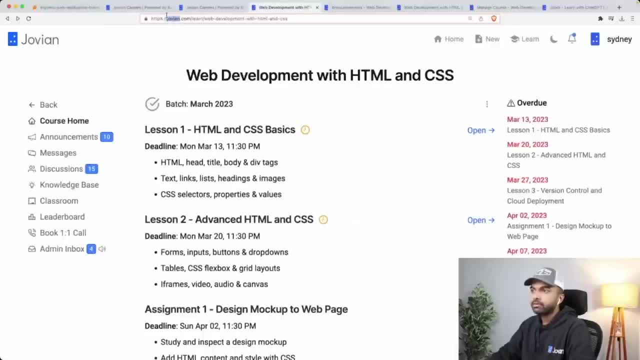 be web pages, images, videos, data, etc. And to communicate with a web server, typically you use an HTTP A protocol, which is where you often see. if you just check the URL of any page, it says HTTPS or HTTP. 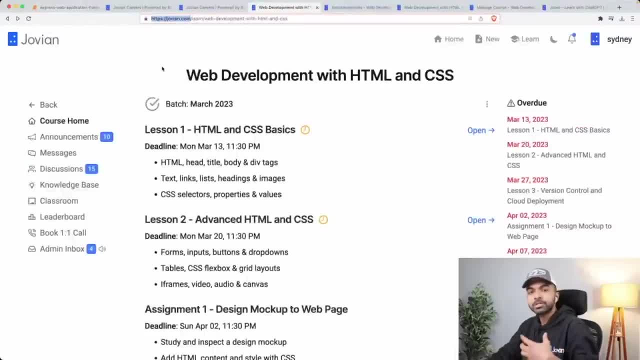 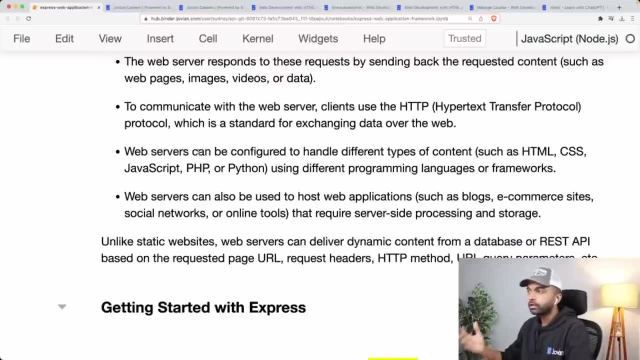 And that basically means that you are using the HTTP. your browser is using the HTTP protocol to communicate with the web server, And web servers can be configured to handle different types of content, For example, HTML, CSS, JavaScript, PHP, Python. all it just depends on what kind of software. 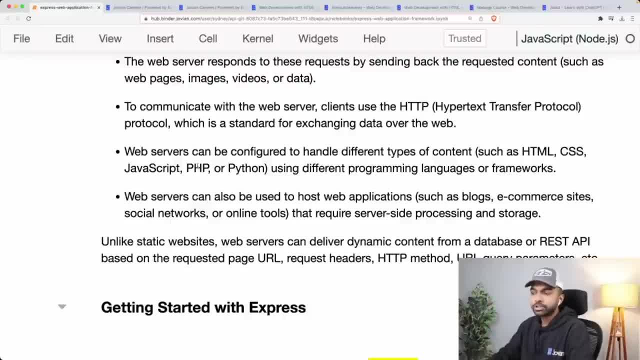 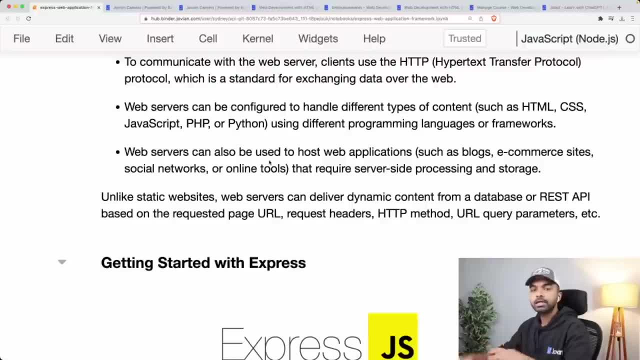 you want to run on your cloud computer which is powering the web server, And web servers can obviously be used to host web applications, For example Jupyter. what we are using here is running on a web server- Jovian itself runs. 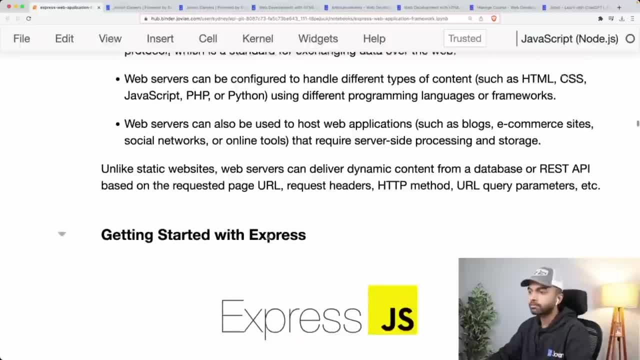 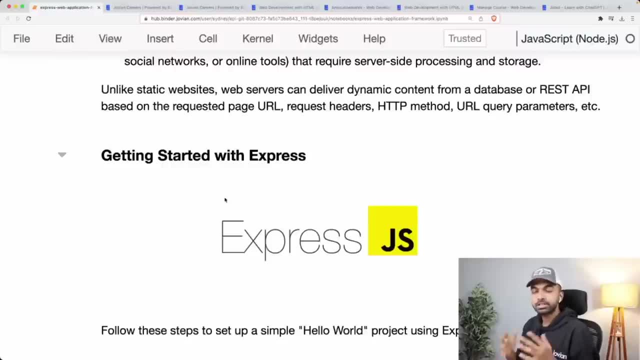 on a web server. Google, Instagram, Facebook- everything runs on a web server. Now, the difference between websites that we've been building today, the difference between websites that we've been building so far, called static websites, and web servers, is that web servers can deliver dynamic content from a database or a REST API, whereas static 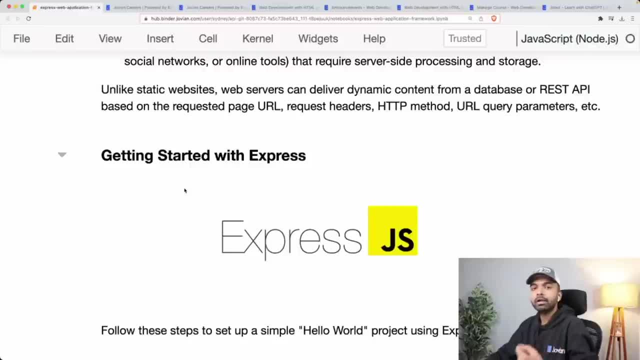 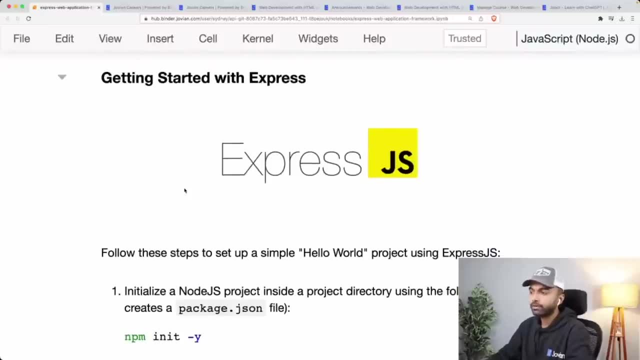 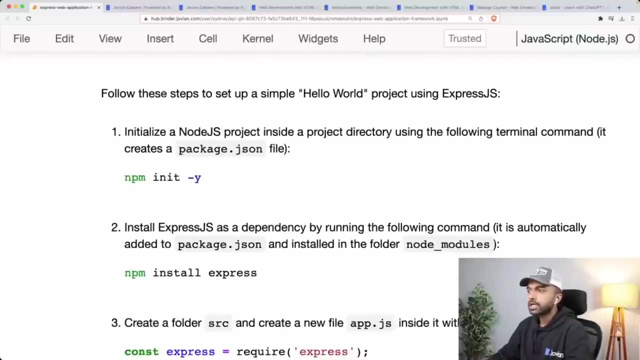 sites like indexhtml, the web pages that we were building, Cannot deliver dynamic content. So today we'll talk about how we can deliver dynamic content using the express web application framework. So let's get started with express. So here's what you need to do to set up a simple hello world project using expressjs. 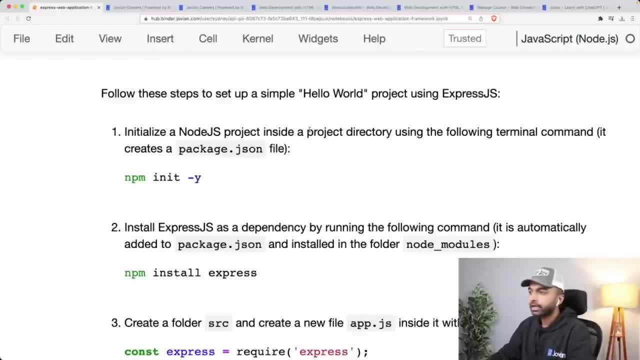 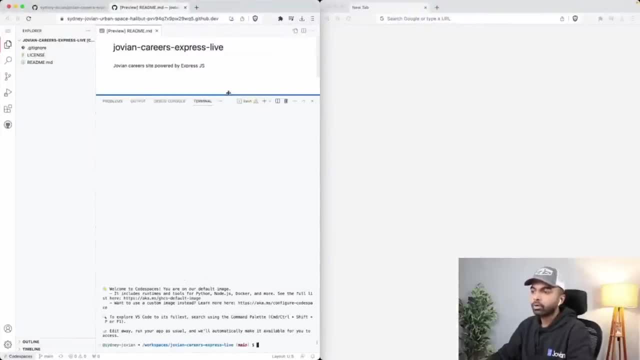 Step one is to initialize a nodejs project inside a project directory. So we are here in this GitHub project, GitHub repository that is open on code space, And I guess we can just go ahead and use this as our project directory. So I'm going to initialize a new nodejs project here. 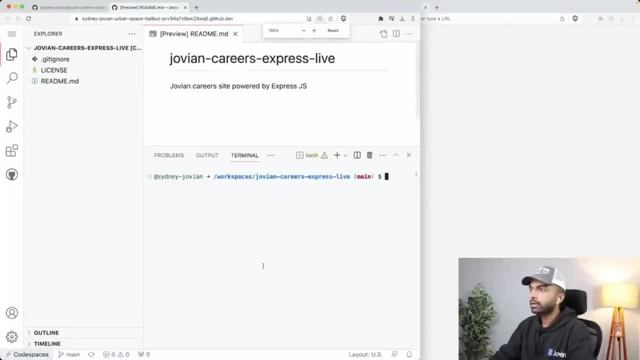 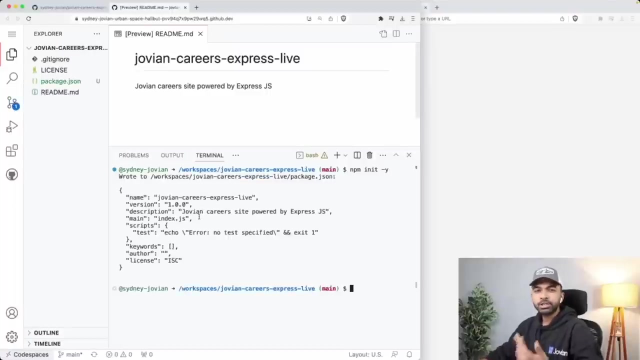 And to do that, I'm just first going to zoom in a little bit, All right. so let's zoom in here, And I am going to start by typing npm init minus y. So let's type npm init minus y, And now you will see here that a project has been initialized. 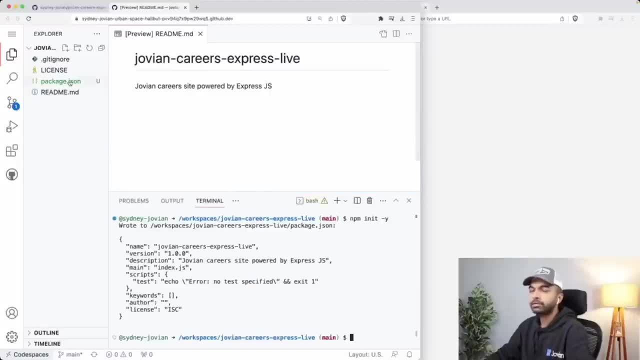 And what that really means is a packagejson file has been created So you can check. here In the sidebar. there is a packagejson file which contains the name of the project, which is auto-inferred from the name of the directory. 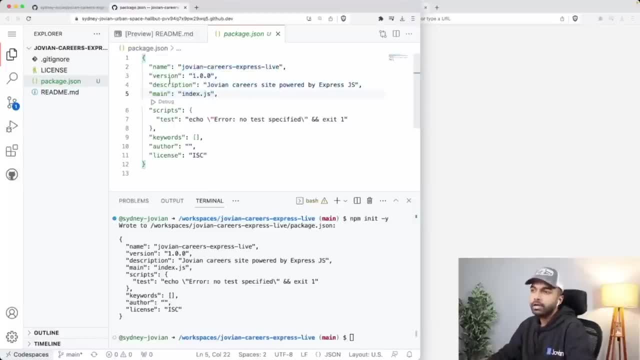 It contains a version and a description. Again, both of these are auto-inferred. Version is set to 1.0 and description is auto-inferred from the readme, And then we have a main file. So this is not something that has been created yet. 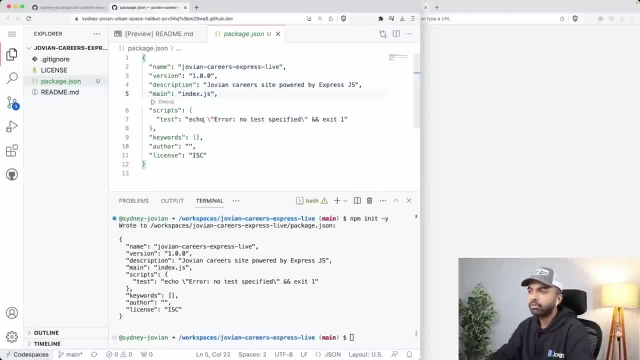 And this is something that we can potentially change when we want to. In fact, we can even remove it if we want. Then we have some scripts here, some keywords, some authors, some license. These are not important right now. These are more. 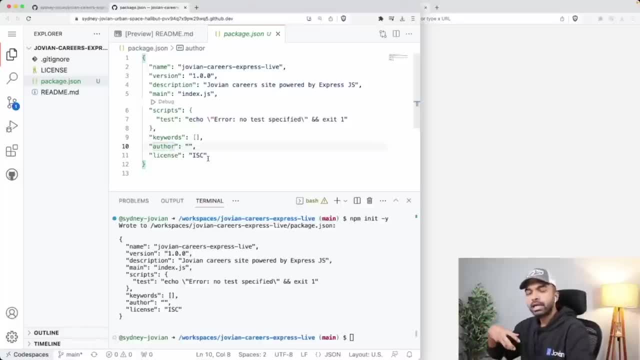 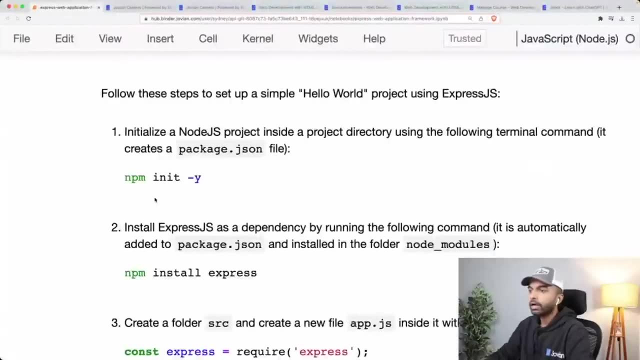 Important when you are publishing a module to the npm registry, But for us, the key things here are these, And these are some things that we will modify over time. All right, So now that we've initialized the Nodejs project, the next step is to install the Expressjs web framework. 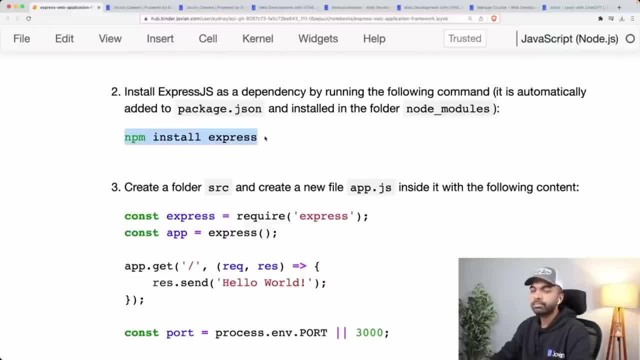 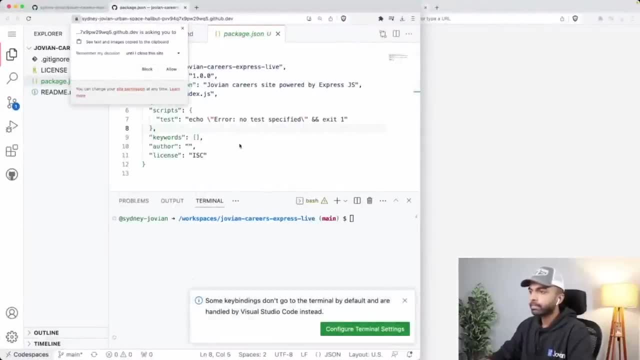 And we're going to install the Expressjs web framework by simply running npm install express. So I'm going to come in here And once again, let me reset things here- And I'm going to say: And I'm going to say: npm install express. 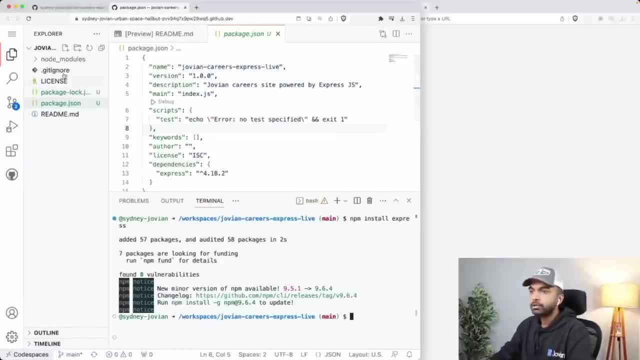 Now, when we click npm, when we type npm, install express, you can see that a node modules folder is created here And inside these node modules folder, express and all of its transitive dependencies get installed. So you can see here that you have you have express here. of course. this is the express framework. 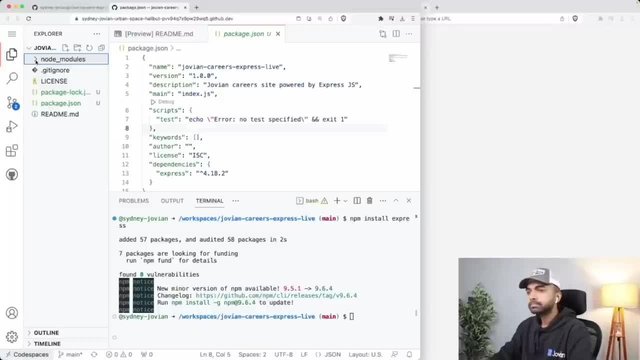 Then there is also a bunch of other frameworks that have been installed. Now I don't want to mention that the node modules folder Will not get added to your GitHub repository when you push these changes back to GitHub, because if you check the gitignore file, you'll see that node modules is mentioned here. 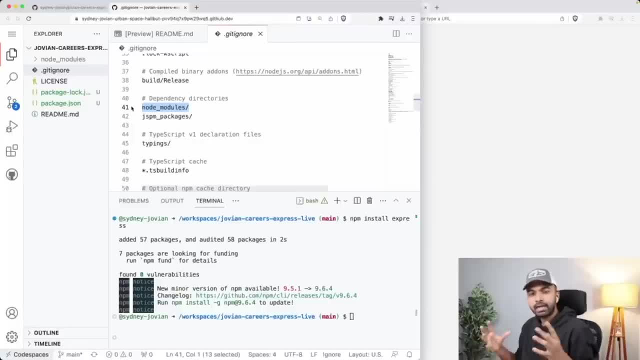 So, basically, we don't want to send all of these dependency files, all that JavaScript code, to our GitHub repository, because that's going to make our GitHub repository really heavy. So instead, what we do is we simply add that dependency in packagejson. 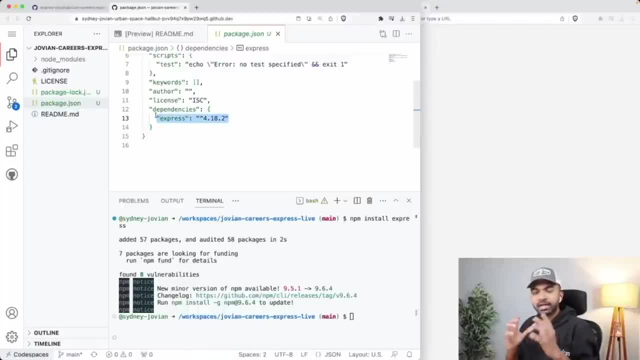 And that happens when you run npm install. So you can see that packagejson contains the name of The dependency that you need to install and the version of the dependency. And whenever you need, whenever somebody, someone else needs to run your code, they can simply get the bare minimum code and then they can run npm install and they can install all the dependencies on their computer. 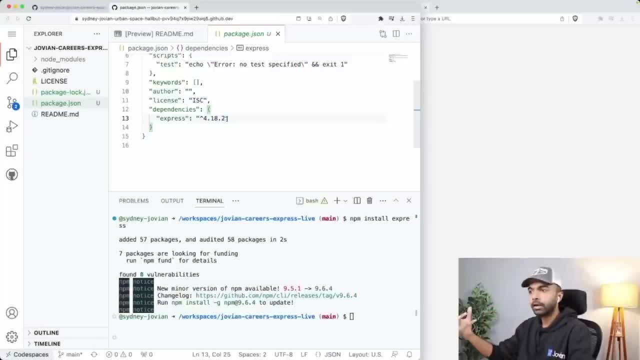 And the same can happen when you're trying to deploy this application to the cloud. All right, So keep that in mind, that we don't commit the node node module server, the node modules folder, to our GitHub repository because it is ignored in the gitignore. 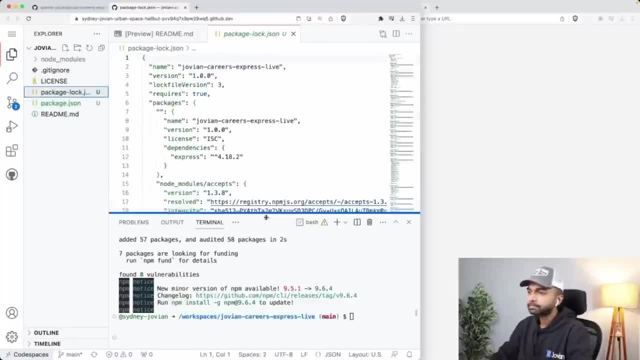 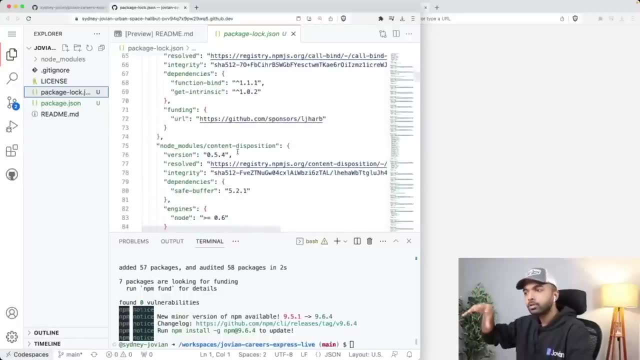 Okay, Now you will also see this package logjson. Basically, what this contains is all the dependencies that node modules, uh, that express JS depends on. those are listed here and their versions are listed here. So this is to ensure that some of the transitive dependencies don't go out of date and cause problems later. 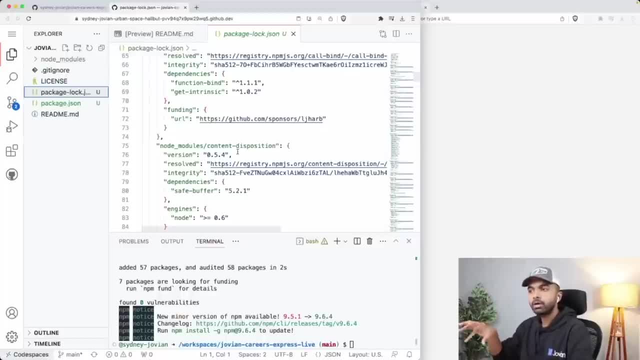 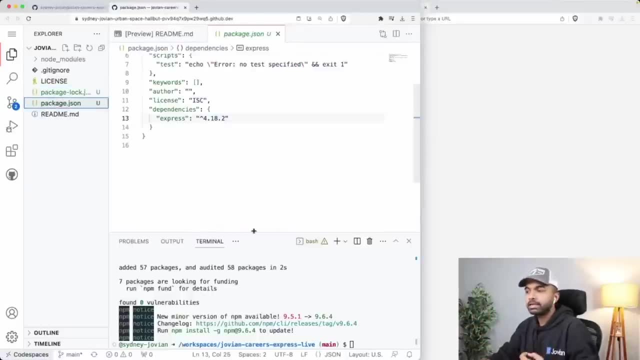 So this is to lock the versions of all the dependencies that you've installed, and and their dependencies, and their dependencies and so on. Okay, Now don't worry if all of that doesn't make sense. The only key thing you should keep in mind is when you say npm, install and type the name of a. 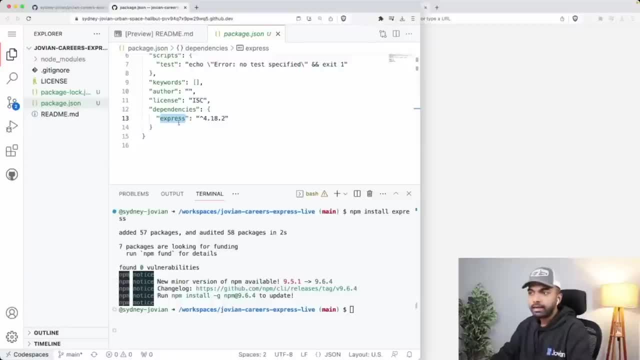 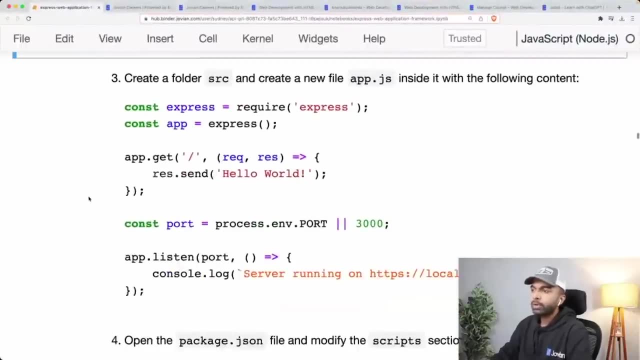 Package that is going to get added into the package, or JSON file, And that can then be used to reinstall that package on any other computer. Okay Now, next, we are going to create a folder called SRC and we are going to put all our application code inside that, all our HTML, CSS, JavaScript, et cetera. 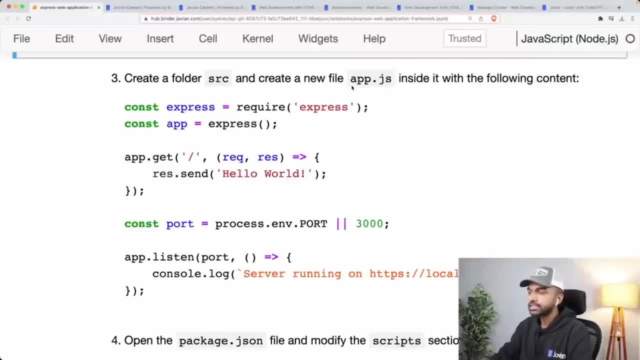 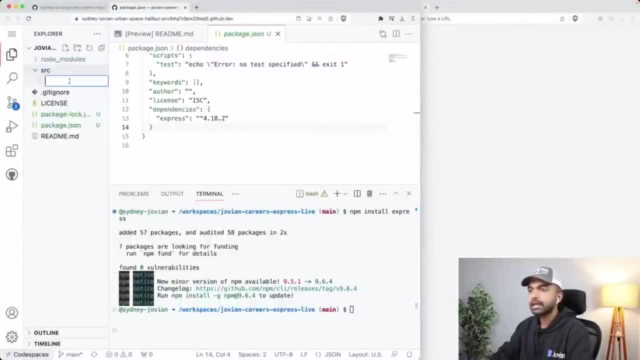 And inside the SRC folder we're going to create a new file, appjs, and inside it we are going to add some content. So let's create a folder SRC. So I've just created a folder SRC And now Let's create a file, appjs. 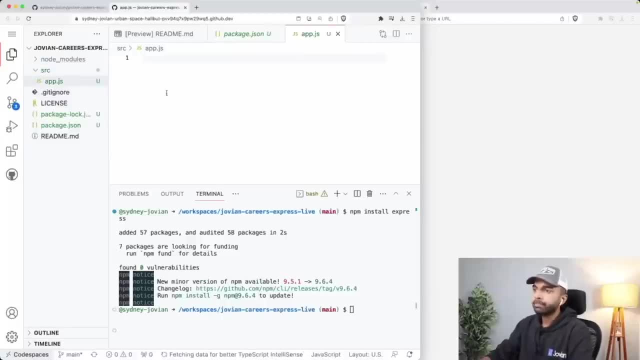 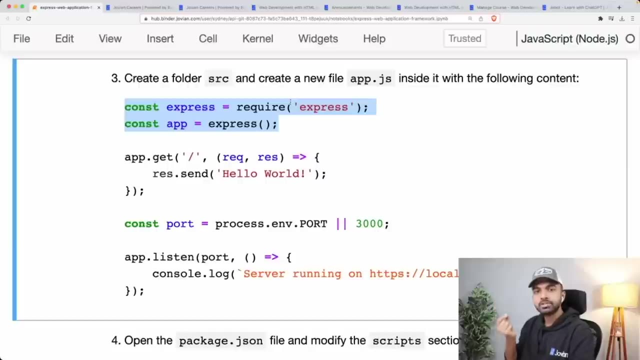 And now in the appjs file I'm going to say: let me copy all the first two lines. So I'm going to say: express equals, require express. This is how we pull in the express dependency. So this is how we get access to the express library: by saying: require express. 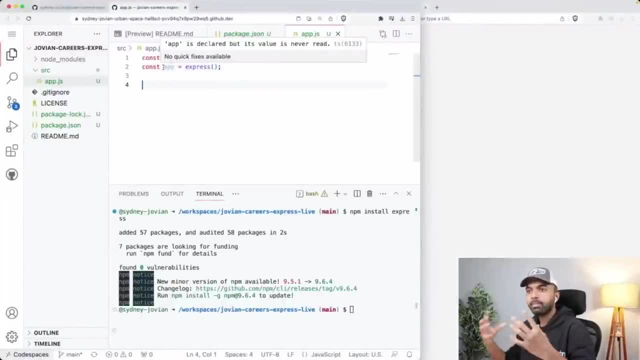 And then I can create an app, an express application, a web application, simply by calling the express function. Okay, And just like that, an app has been created, A web server has been created. But we're going to do a couple more things as well. 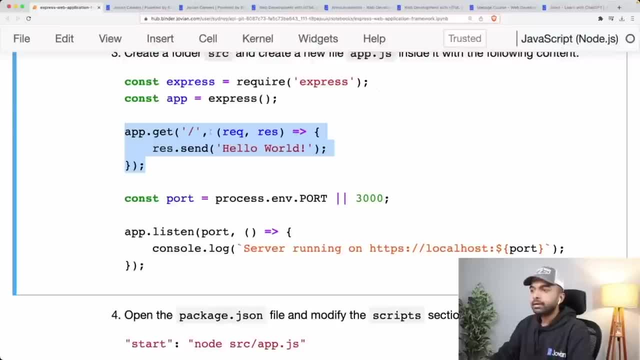 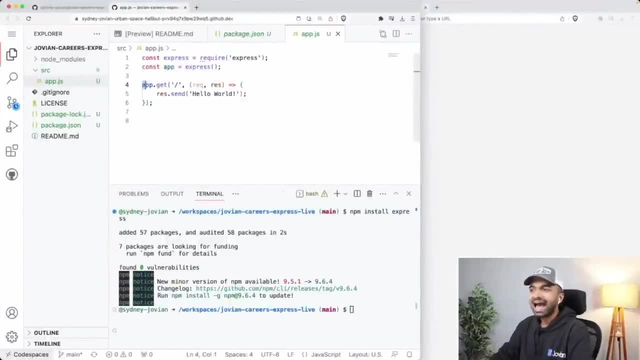 Now the first thing we're going to do is set a basic, um, set us basic route. Okay. So let me just paste this over and then we'll talk about it here. So what we're saying is appget. So we're saying that when the app gets a request and when it gets a request on slash- which means when it gets a request on the basic route- right by the basic route we mean it's simply, let's say, this application was deployed on joviancom. 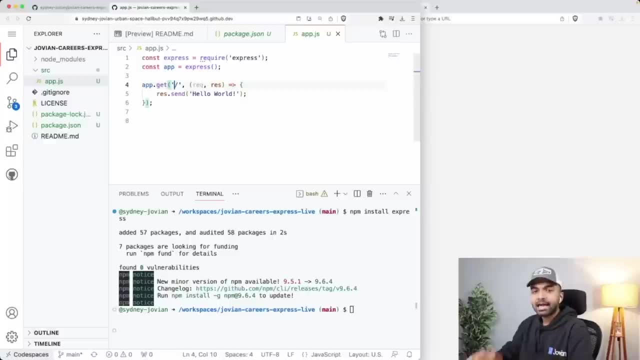 Then when you try to access joviancom, That is treated As the slash or the root level route. But let's say, if you try to access joviancom slash, that would be treated as the slash. Okay, So if you just try to access the server raw, without any sub path to the URL, then that is going to get sent to this particular route. 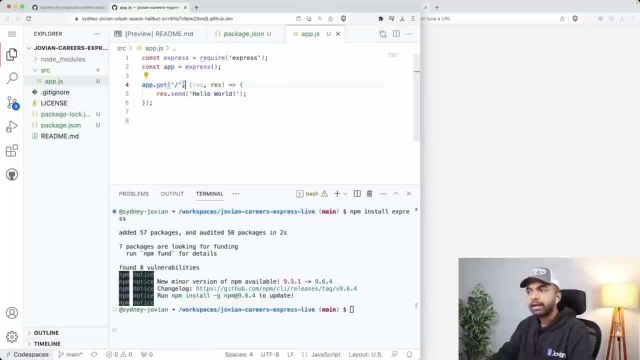 So, whenever you address, whenever you're attaching a route Handler to, whenever you're attaching a route for an express application, you need to specify a route handler, which is basically just a function That is Given the request that has been sent from the client and that is given a response object and it can then use the response object to send the data back to the client. 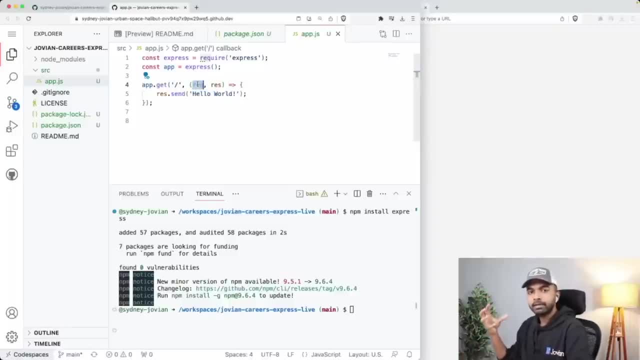 Okay, So the request object is used to get data from the client, The data that the client has sent in this request. the response object is used to send data back to the client. All right, So you will see this pattern very commonly in all JavaScript web frameworks. 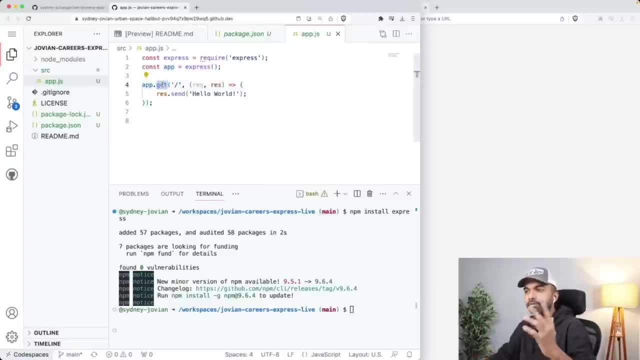 You'll attach a route and the method could be get post et cetera. We'll talk about that, but you'll attach it out And uh to the application And for that route you will specify a route handling function. 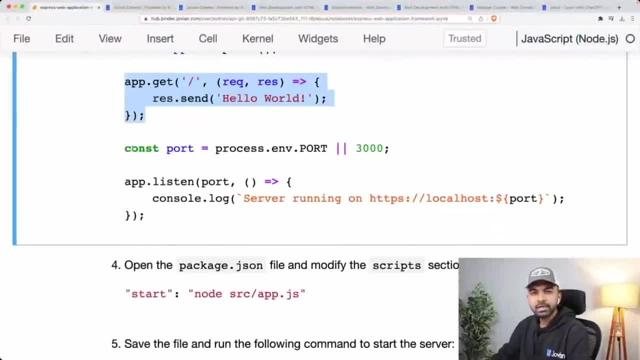 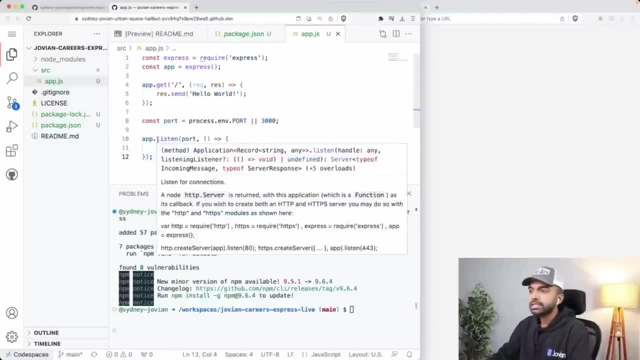 Okay. Finally, we actually need to run the server, and the way you run the server is by calling app dot listen. So once you've created an express application, you can say app dot listen. And basically what this is saying is: now the app will start listening for requests. 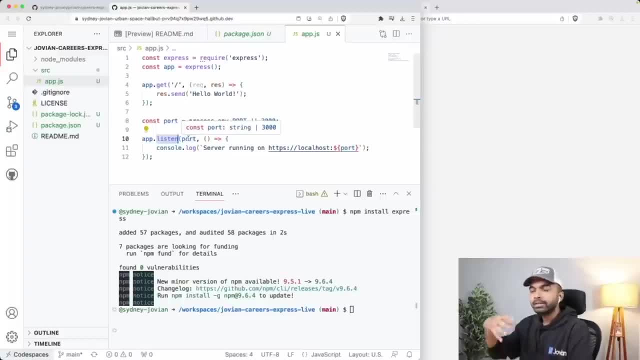 Now, to start listening for requests, it needs to specify a port. There are many applications that can run on the same computer, on the same hardware, So the different applications Or different servers can occupy different ports. They can listen at different ports, All right. 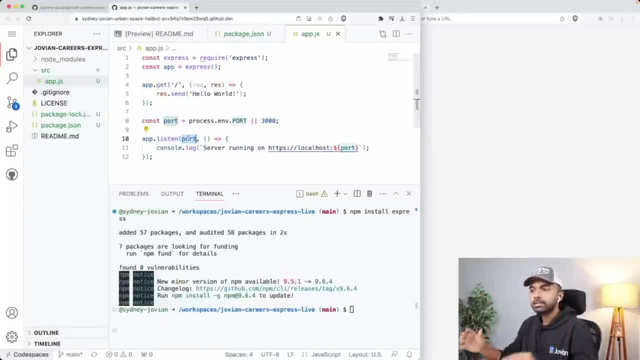 So that's where. so think of it as mailboxes within a building. So you specify your mailbox number or your port number. So let's see, Uh app, dot, listen, port. And the port is currently just being set to 3000, but what we also often do is sometimes, while running, the application of an external port is specified. 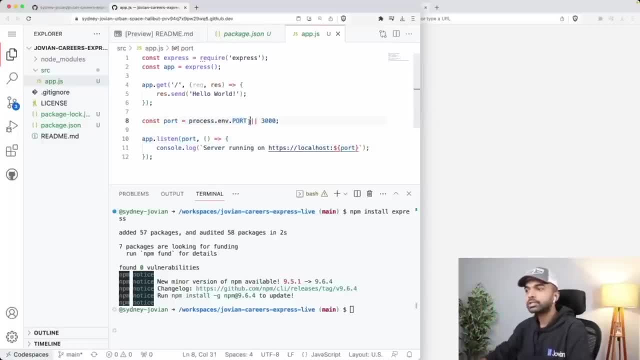 So when an external port is specified, while running the application that is going to be created, It's going to be configured in what's called an environment variable process, dot E and V dot port. But we uh, if that is not specified, we just pick the default value of 3000.. 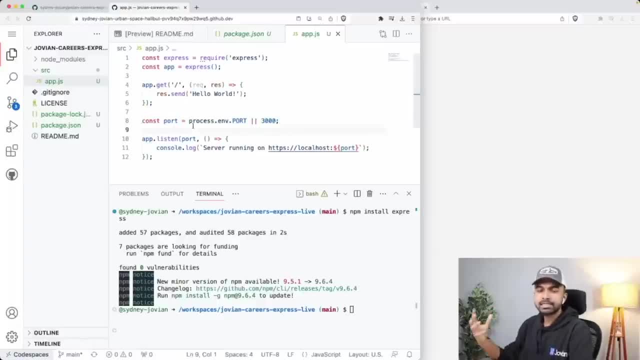 Okay, So far. now again, don't worry about this line. Basically, what it says is use the port 3000. If no other port has been specified while running the application. Okay, All right, So this app is going to start listening on the sport 3000 when we run the project. 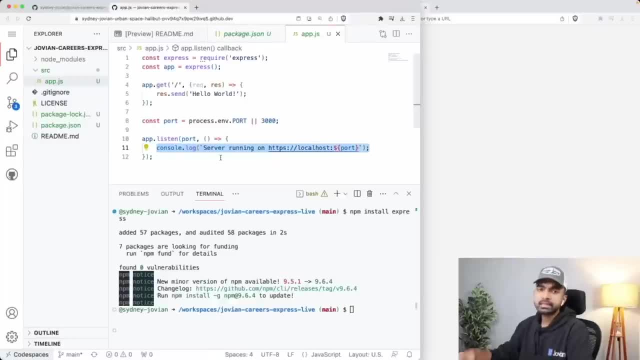 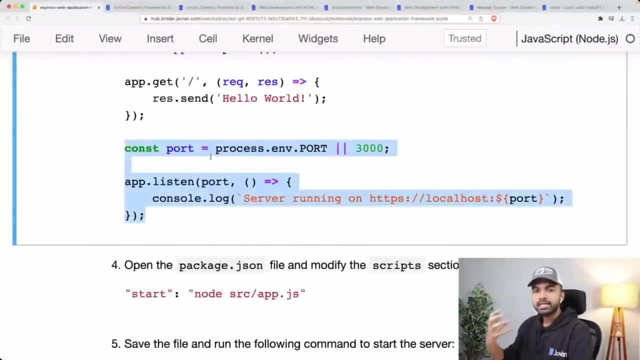 And it is also going to just print something out to this, uh, to the console, saying that the server is running on such and such URL. Okay, So with that we have set up our very basic web application that is going to take a request and simply return. hello world. 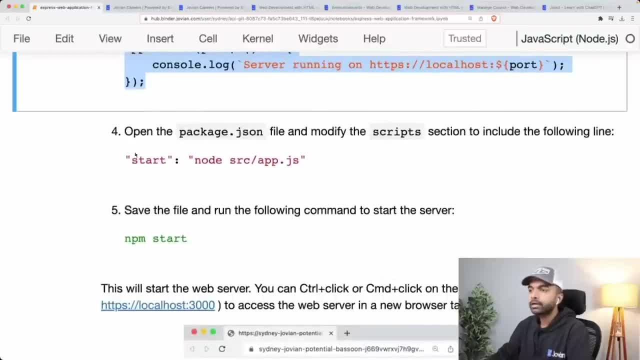 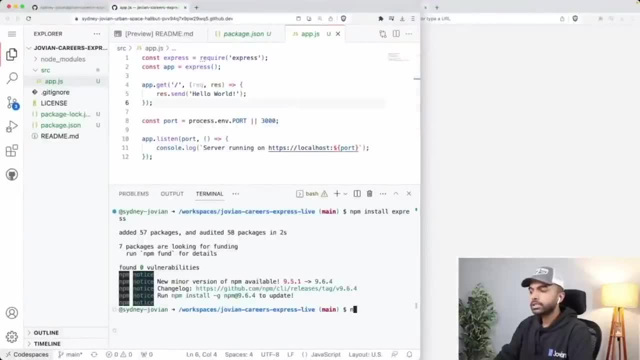 Now, uh, the last thing we need to do is we actually need to configure um command to run this server. So one way we could run the server is just go and say: node, SRC, slash, app, dot, JS. Okay, That's one way to do it. 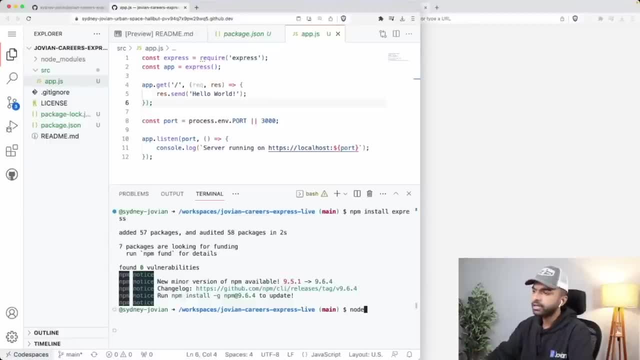 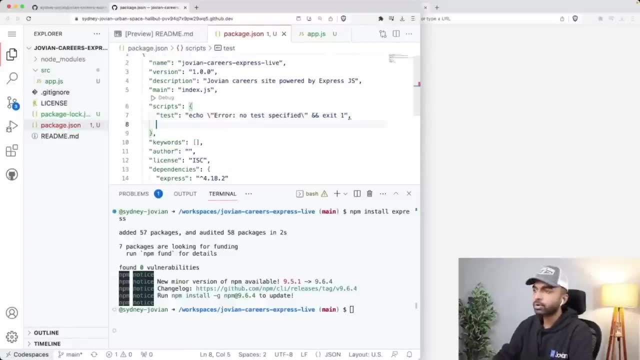 We just go into the terminal and type node SRC, slash, app, dot JS. but the preferred way to run it And or configure applications in general is to specify the script that is used to run the server in the package or JSON file. So in package or JSON you will, you will have this scripts object. 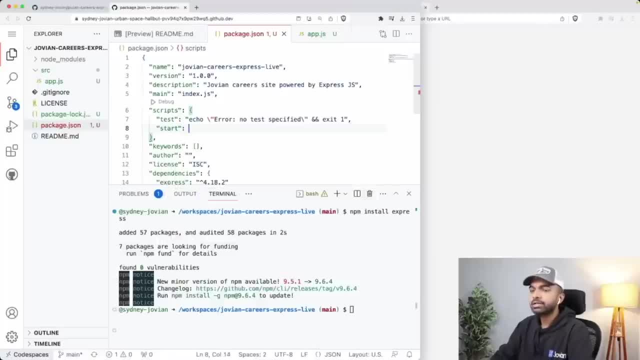 And in this scripts object, it is common to just add a start key And in that start key specify what command should be executed to start this application. Okay, And the command, of course, that we want to execute as node: SRC slash app, dot JS. 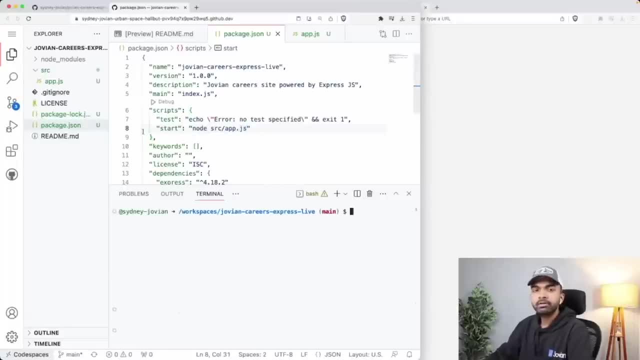 Okay. So now that we have done that, now that we've started, now that you have specified a start script in um package or JSON, we can say NPM run, start, Okay. And when we say NPM run start, that is going to do the exact same thing as node SRC slash app dot JS. 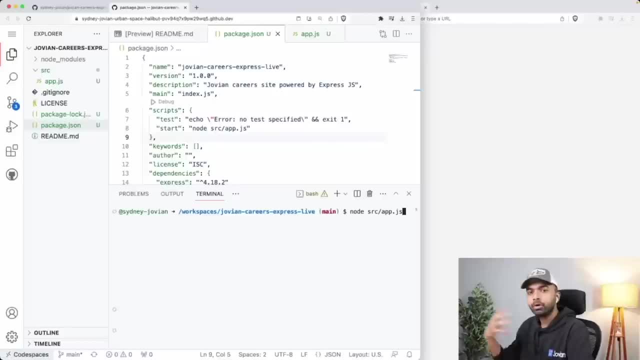 Why are we doing NPM run start? Well, it's just good convention. any node JS applications that you create, it's a good convention to specify the start script so that somebody else who's running the application can does not have to guess what the start script is going to be. 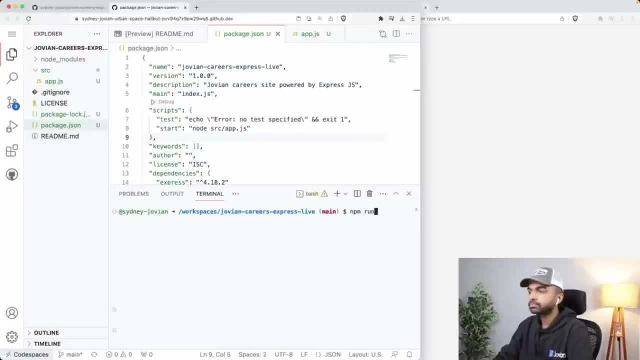 Okay, So let's just Run NPM, run start, And with that the server is running. So now the server is running on the visual studio code. Uh, the server is running on the GitHub code space machine that is somewhere in the cloud, and to access that machine we can just click this open in browser button that shows up. 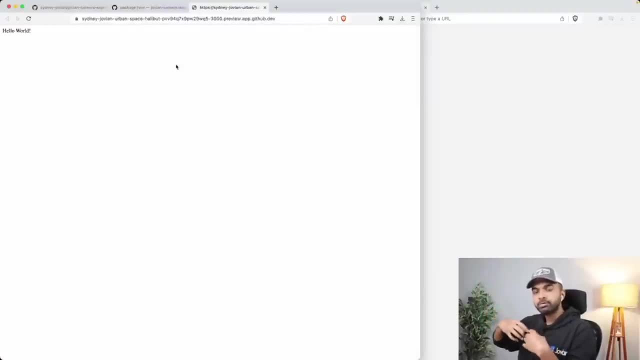 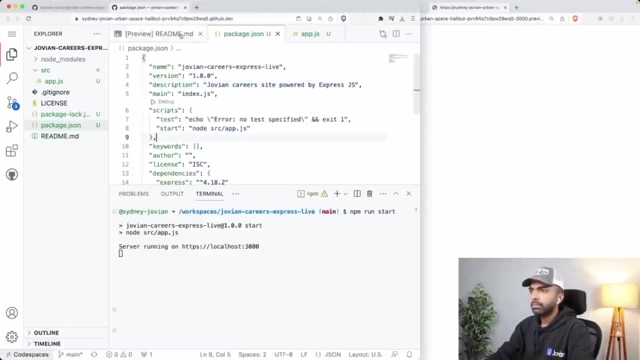 What it does is, that is, it takes our request from our browser and forwards it to the port number three, 3000 of the GitHub code spaces machine. Okay, And you can already see here we now have on this port we are simply printing hello world. and you can see now that if I just changed this to hello Jovian and I kill the server and I restart the server and I reload the space, you can see now it says hello Jovian. 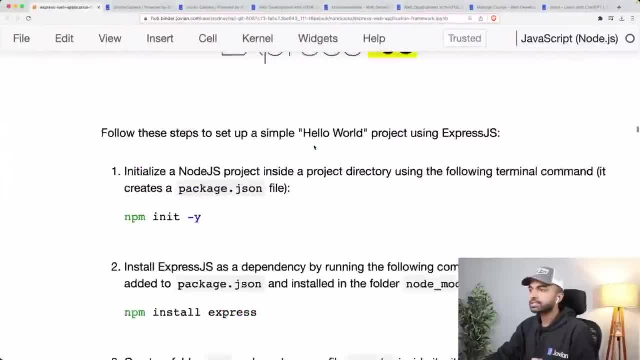 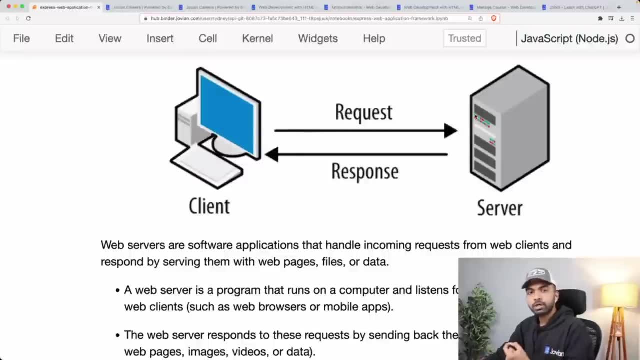 So, just like that, we have set up our first basic server. So here's what's happening: when we type the URL into the browser, that URL sends a request. Okay, Okay, Okay, Okay. So we have sent a request to the server and see this URL. 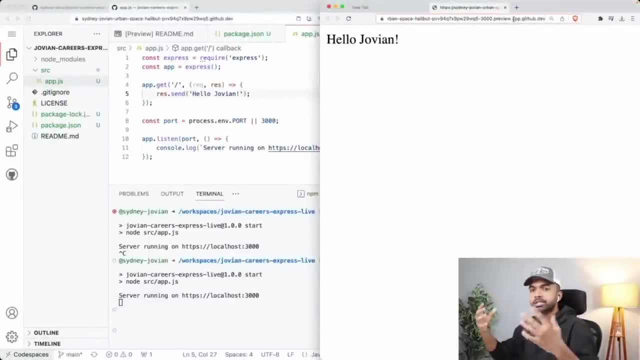 This is basically just like a simple URL, like a simple something or somethingcom, ordev slash, and there's nothing after it, And that is why that is going to match with this particular route handler, And this particular route handler simply says: hello, Jovian. 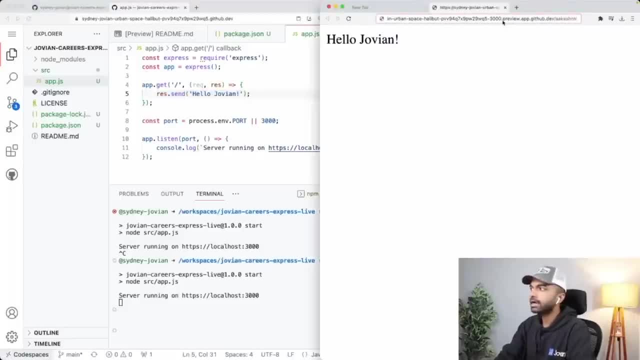 Now suppose I had said here: slash Akash NS. So if I had something at the end of the URL, slash something. you can see that it says cannot get slash Akash NS. It only knows how to get slash, And we'll see how to add more of these routes to our server. 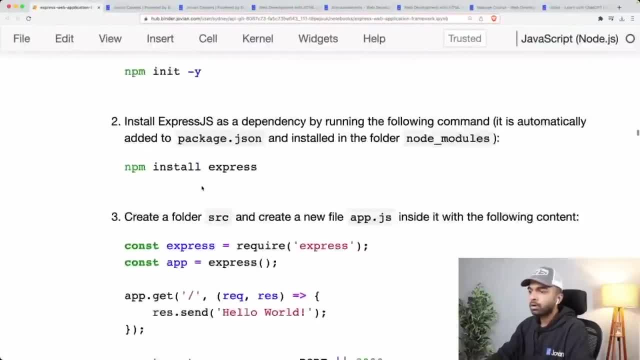 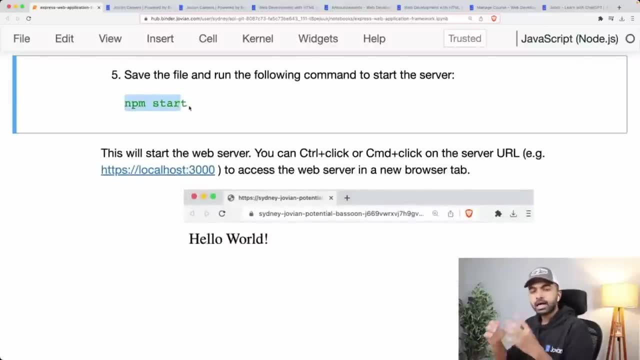 So we'll see how to add more of these routes to our server shortly as well. Okay, So now we've set up our dev server, And one thing I want to mention is, instead of running NPM run start- because start is such a special common command- you can also just say NPM start instead of NPM run start, and both do the same thing. 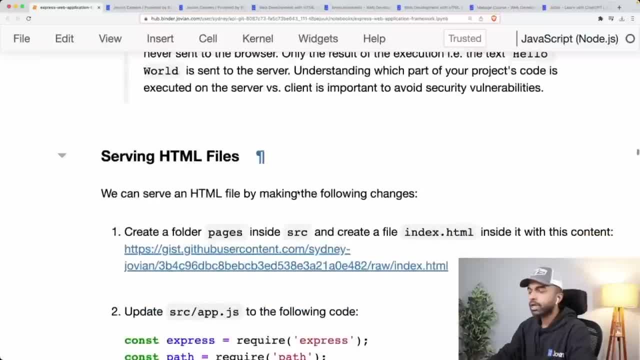 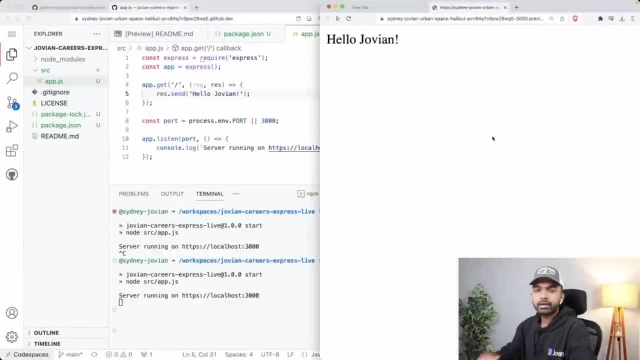 And with that we have set up a web server that shows hello world. Okay, Now the next step would be to serve an HTML file. Now, of course, we don't just want to return hello world from our server, We want to actually return some nice HTML. 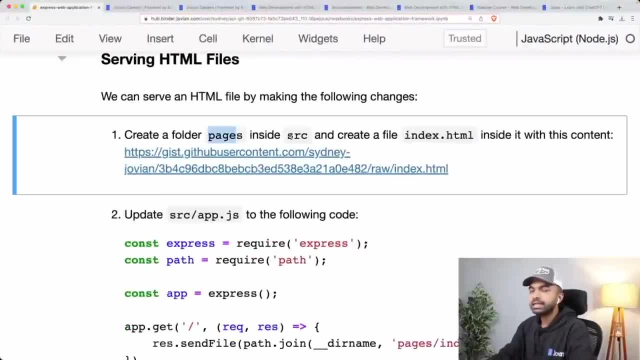 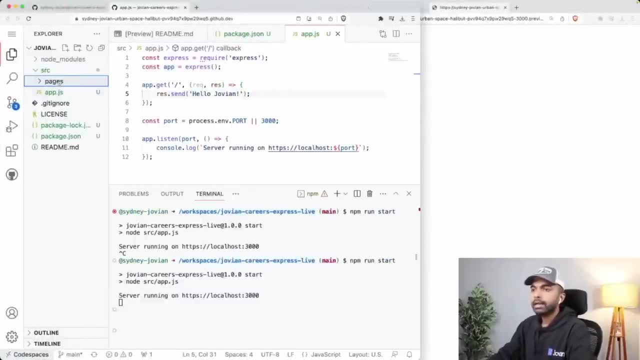 So here's what we'll do. We will create a folder pages inside the SRC folder. So I'm going to say SRC, I am going to create a new folder pages, All right, And now inside pages, I'm going to create a file index dot HTML. 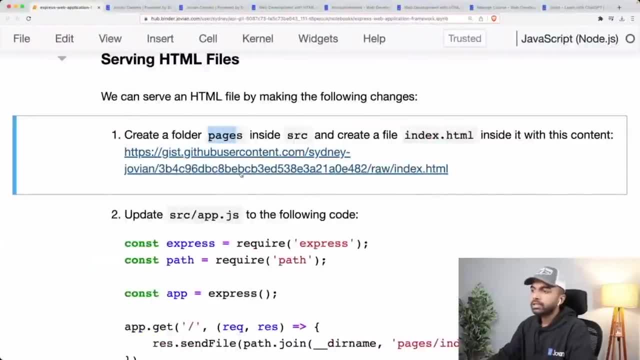 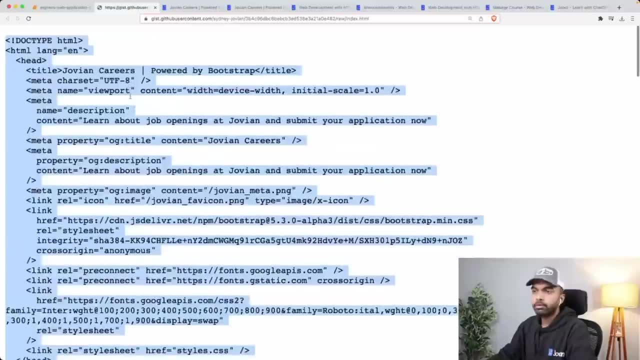 So now we have an index or HTML file, All right, And into this index or HTML file I'm going to put in some content. So I'm just I've just taken some of the content from the, from the, A website that we had created the last time, the Jovian careers website, and I 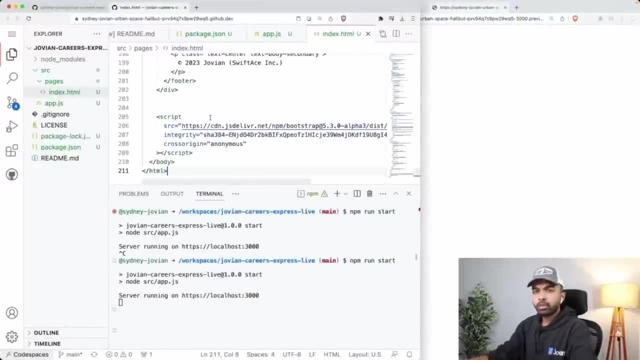 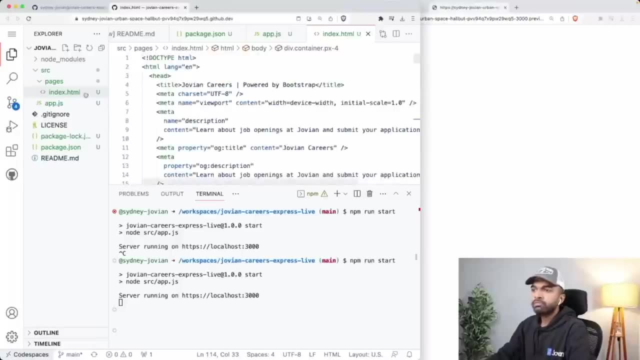 have included it here on this link, So I'm just going to copy paste it, because we don't want to just sit and reimplement the entire piece that we had created the last time already. Okay, So now we have put in inside SRC, we put in a folder pages and inside pages. 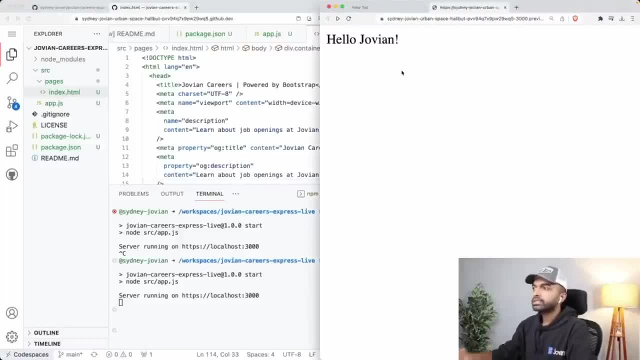 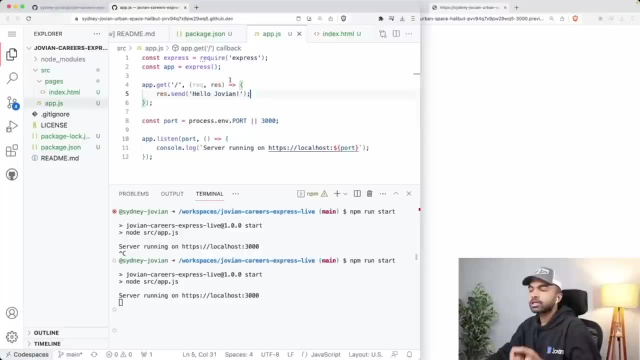 we put in the file index or HTML. However, this browser has no way to actually access that index or HTML file. This browser can only make a request to the server And the server is only listening on the route slash and on that slash route. 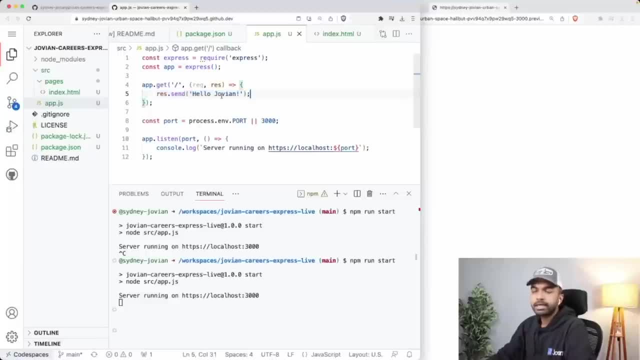 it is simply returning hello Jovian. It is simply sending hello Jovian. So, instead of sending hello Jovian, we need to send the contents of the index dot HTML file. All right, How do we do that? Well, here is what we can do. 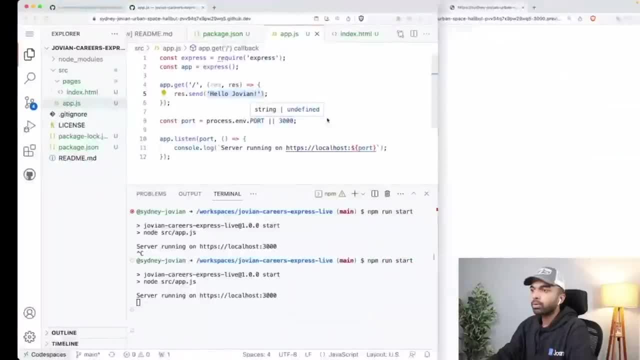 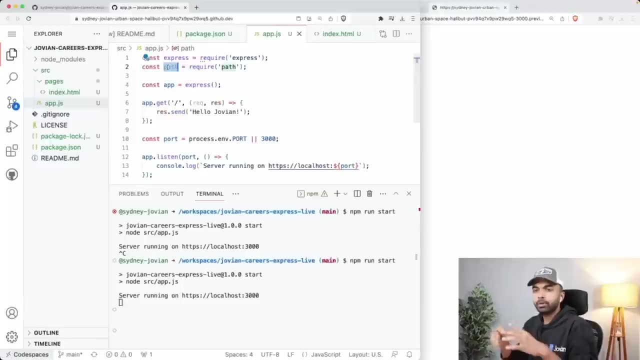 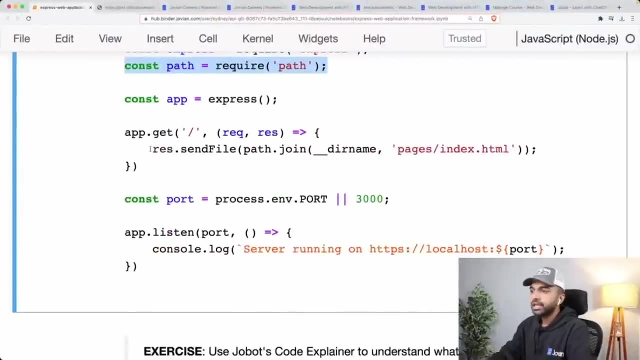 So we can first include this new utility function called path. So we say path equals require, require path. And this is path is simply a utility to construct Full file system paths based on, based on relative paths. Next, let us change this one line of code. 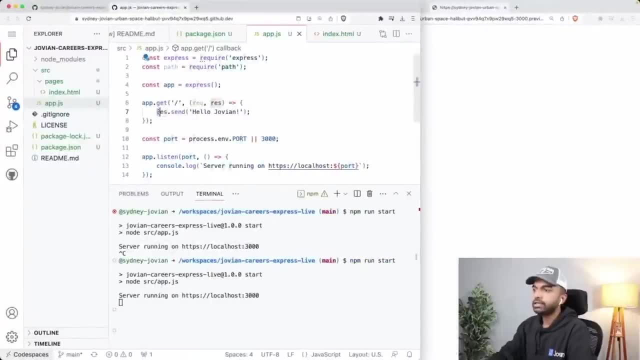 So instead of saying rest dot send file, instead of saying rest dot send hello Jovian. so let me comment that out- I'm going to say rest dot send file. path dot join der name. Der name is basically just the name of the current directory, which is dot slash, SRC. 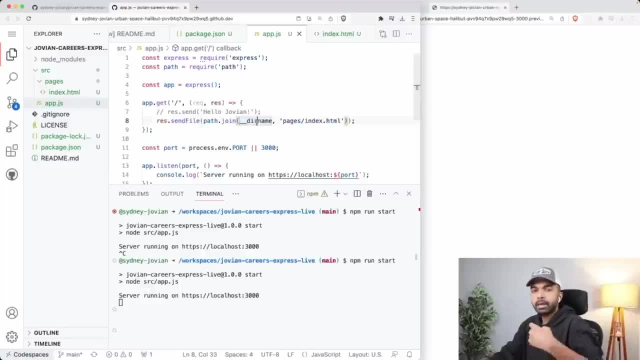 So underscore. underscore der name is a existing variable in nodejs that automatically gets the name: Name of the current directory. So you want to take the name of the current directory and to it we want to join pages. slash, index dot HTML. All right. 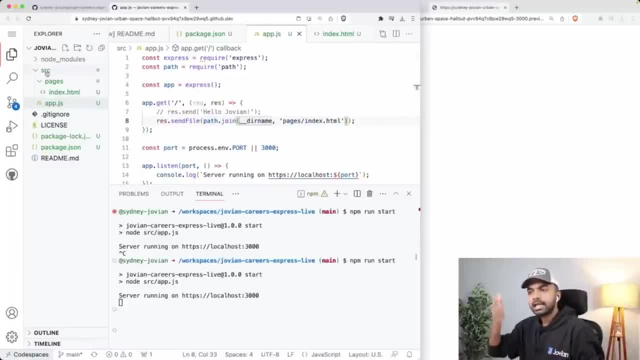 So we want to get current directory, which is the SRC folder, slash pages, slash index dot HTML, And we want to send that file in the response. All right, That's all we are doing here. So let us hit save again and let us reload the page. 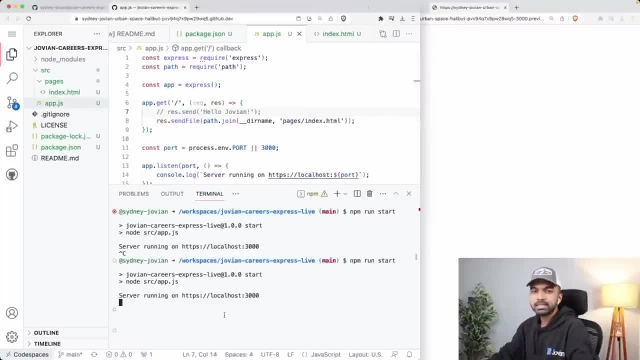 Nothing happens because we have to restart the server. So remember this express. what it does is, when you start the server, it reads the entire JavaScript file And then, if you make changes, you have to restart the server. So let's see controls. 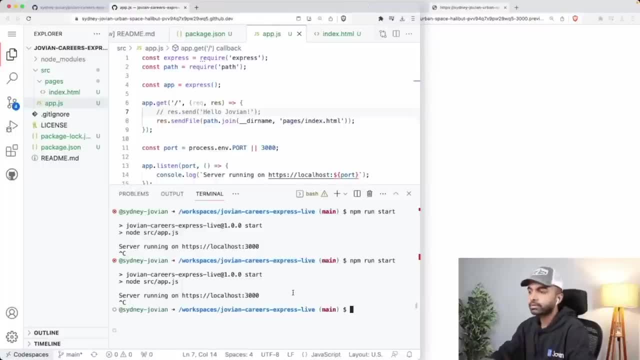 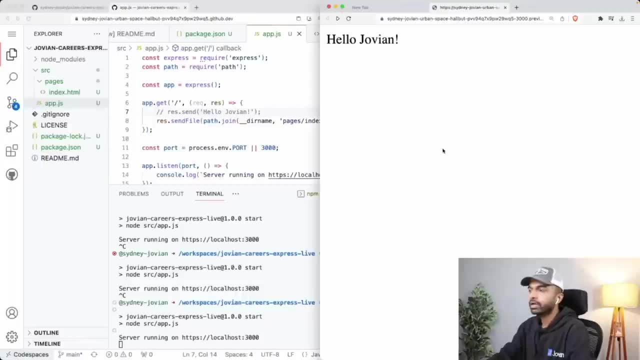 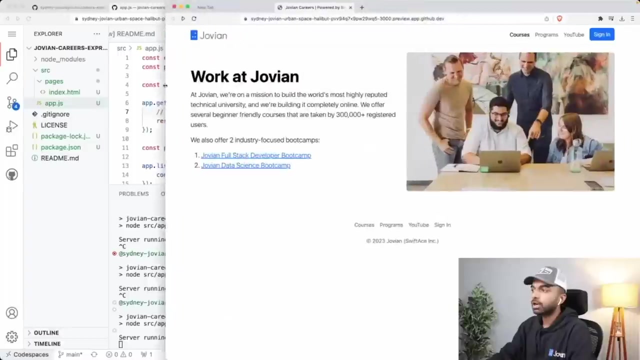 Let's type control C. control C is used to kill the server or stop the server. And then so you just go into the terminal, press control C and then type NPM run- start or NPM start again. And now, if we reload the page, you can see now that it actually shows us the job. 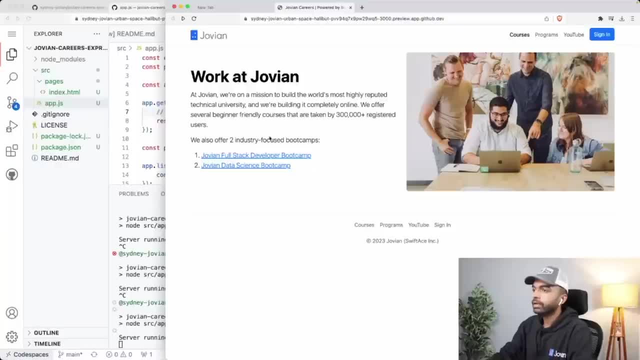 applications page that we had created earlier. So it has a header, It has this work at Jovian over here And it has This footer over here as well. All right, We've not added the jobs table and we've not added the application form yet. 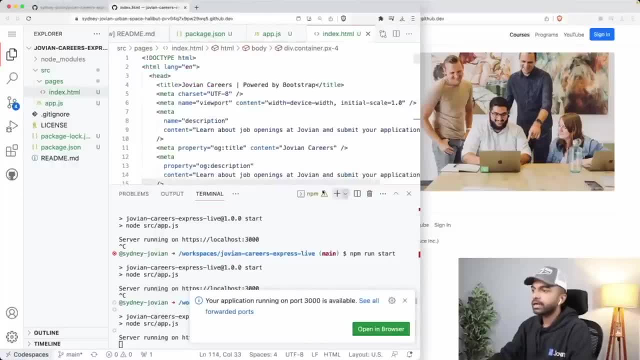 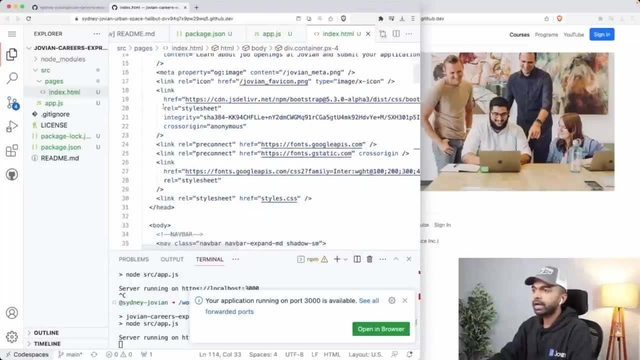 We've just added these parts and you can, of course, you can study the code inside index dot HTML to make sure that's exactly what we have. So, yeah, we have a head and inside the head we have a title, We have some meta tags. 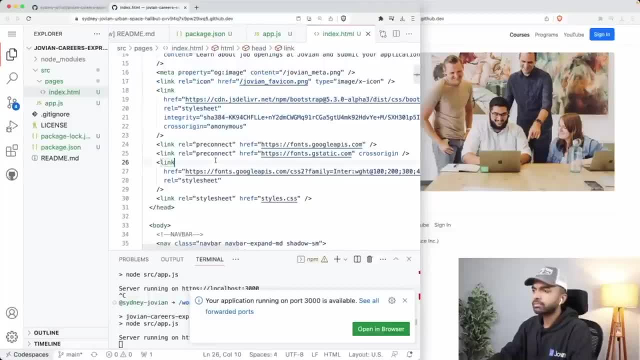 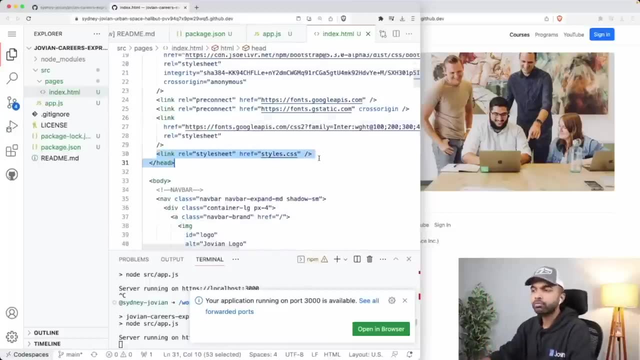 It looks like we have some link tags: Jovian favicon dot PNG. We have some um, we have bootstrap, we have some fonts and it looks like we have a style sheet- styles dot CSS. So we might need to add a few more files. 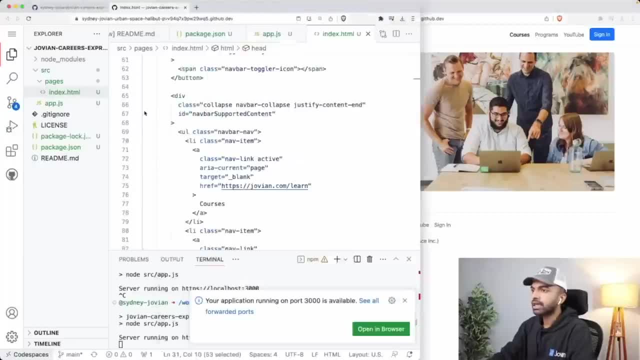 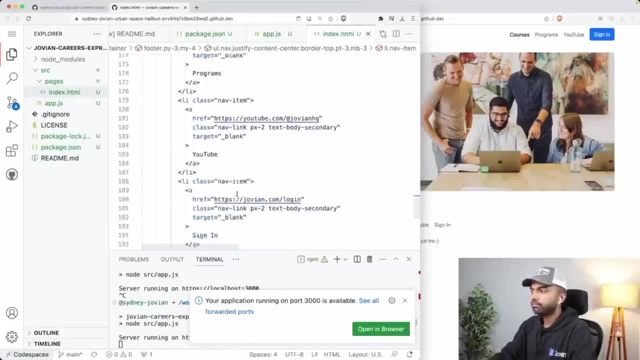 But then we have a nav bar over here and that is what is showing this nav bar. Then below the nav bar we have this about Jovian section over here, All right. And then below the about Jovian section, we have a footer over here and that's. 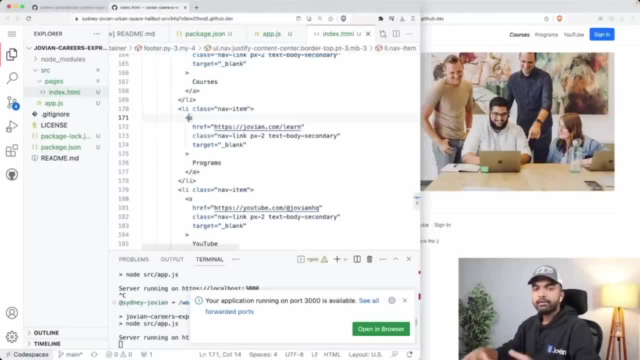 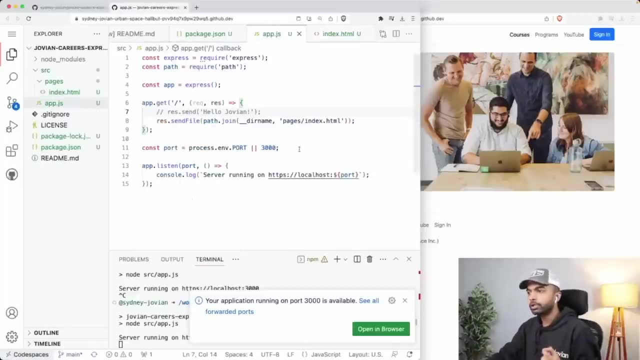 basically what we are showing on the page. All right, So with that, we have just returned some HTML from the server. Now, one very important piece of information I want to point out to you- to you here- is to understand what is visible on the server and what is visible. 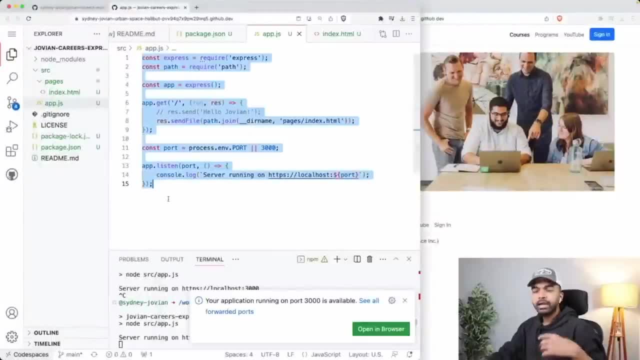 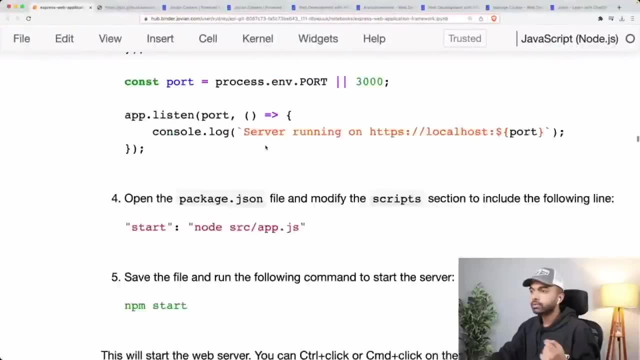 on the client. Now, all of this code that we are seeing here, it is JavaScript code, but this JavaScript code is not running in your browser. This JavaScript code is running on the server. So your browser simply makes a request, Your browser simply sends a request to the server. 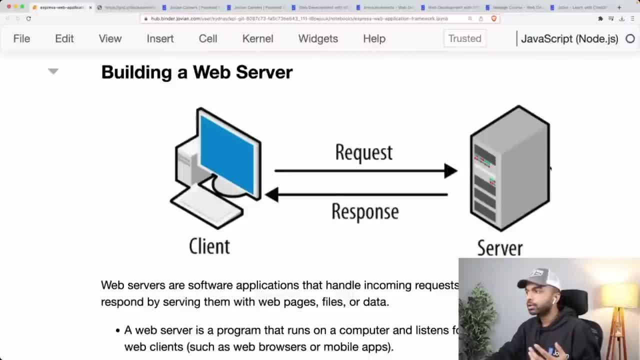 All the JavaScript code inside appjs is executed on the server, It picks up the indexhtml file and it sends it back to the browser, And now it's in the browser that the indexhtml file is parsed and displayed as As a webpage. 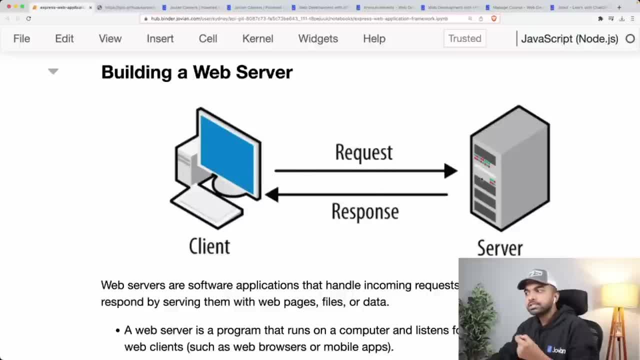 Okay. Now what you might also have is that you might also send a JavaScript file to the server, to the browser, and then that JavaScript file can get executed on the browser, on the browser as well. Okay, But that's different from the appjs file. 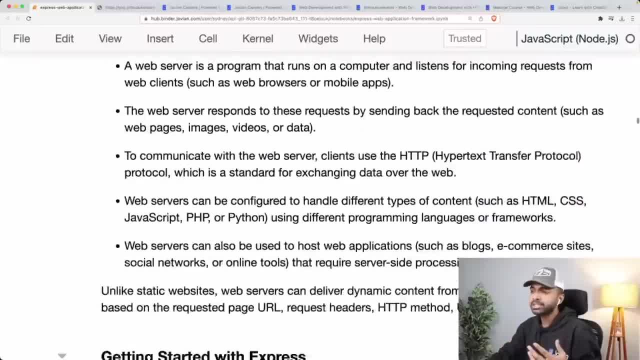 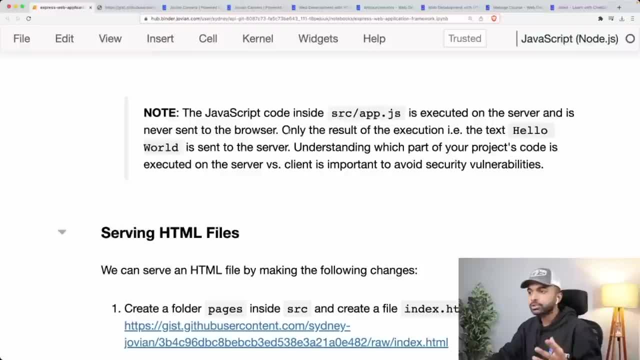 The appjs file only runs on the server, And I'm stressing this again because this is a common source of vulnerability, right? So understand that only the result of the execution, which is hello world, or the HTML file, is sent to the browser. 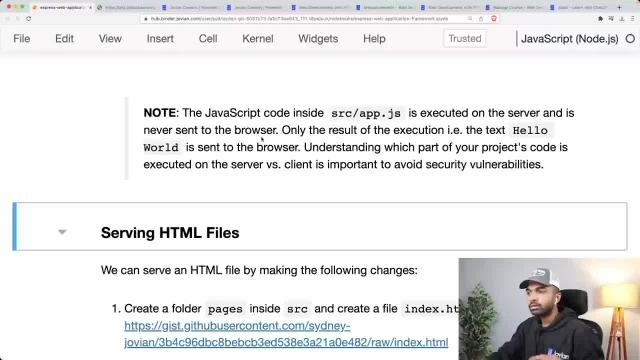 They should say browser. It's sent to the browser and the rest of the code remains on the server. So understanding which part of your project code is executed on the server and which part of your project code is executed on the browser is very important to avoid any security. vulnerabilities. You do not accidentally want to send some database credentials to the browser, because then your user will be able to see your database credentials and they'll be able to access your entire database. Rather, you want to keep them on the server and just send the response that the user needs. 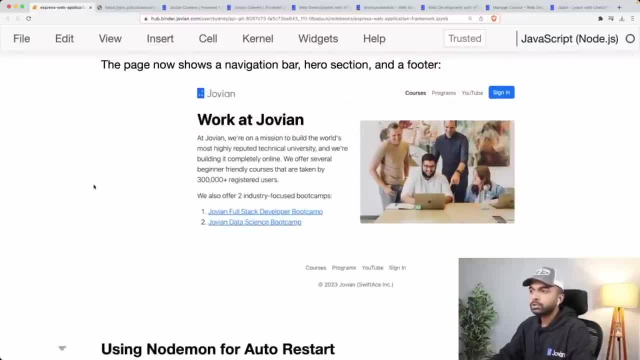 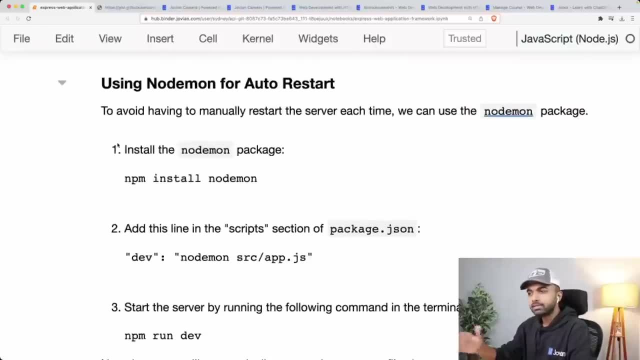 to them. Okay, So with that we have figured out how to display a HTML file, So that's great. Now the next step is to maybe make our workflow a little easier. Every time we make a change to the index or HTML file, we have to manually restart the 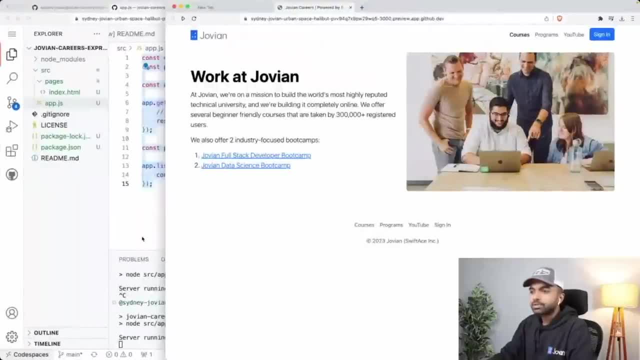 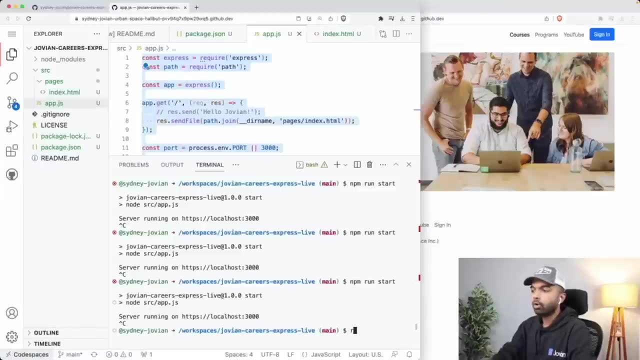 server And each time that requires us to go in press control C and then restart the server. There's a better way to do this. There is this helper library called node mon, which stands for node monitor. So I'm just going to say: 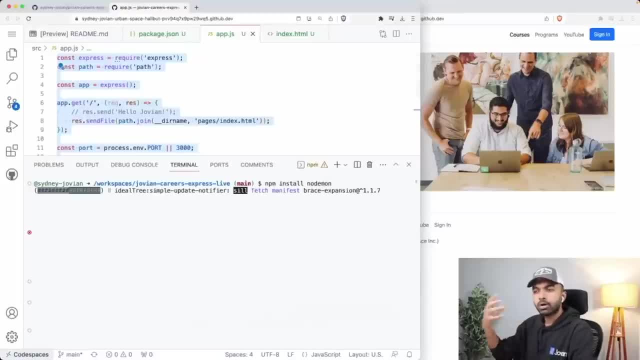 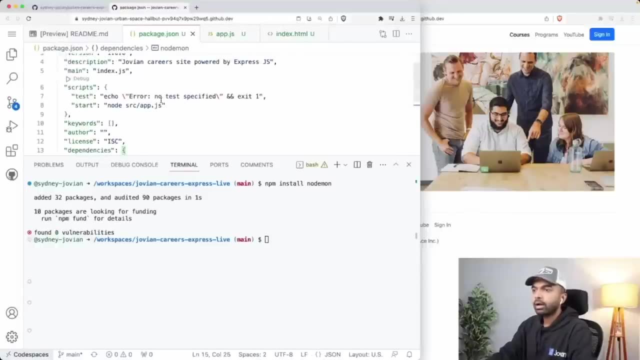 NPM: install node mon. So that's going to install the node mon package for us And you can see here that it gets added here to node mon. All right, And now I'm going to add another script here called dev. So now in my package- or, Jason, I already have the NPM start script, which is going to be: 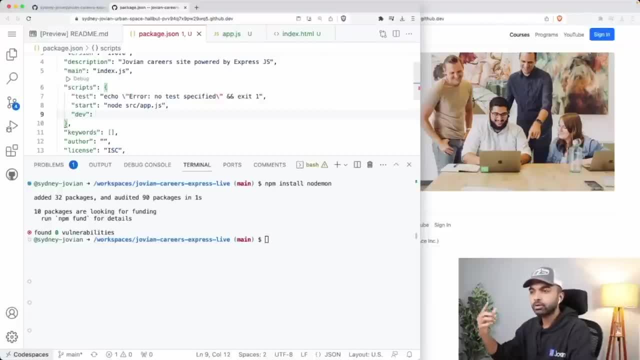 used when I'm happy with all the code, I don't feel a need to change the code too many times. but I also want to use another script during development, And here I'm just going to say node Mon SRC slash appjs. 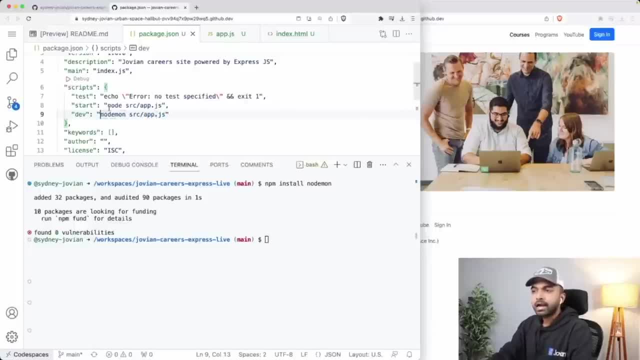 So the only change we've made between start in dev is that start has node SRC slash appjs and dev has node mon SRC slash appjs. What this is going to do is every time the uh, every time there is a change made to any. 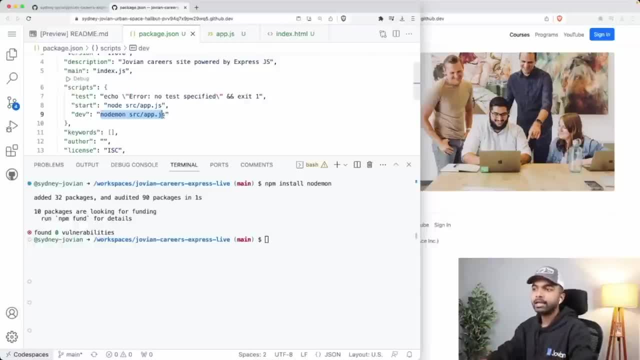 file in the project. it is going to restart the server automatically, so that we don't have to come in and restart the server manually. Okay, So let's now run NPM run dev instead of NPM run start. I'm just going to run NPM run dev. 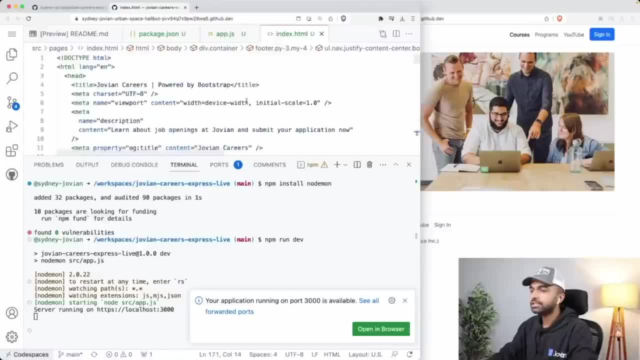 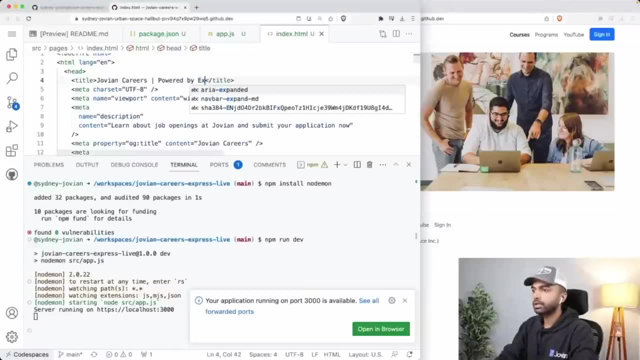 And now You can see that if I go in here and I change the title of this page, for example, so the title of this page is Jovian careers powered by bootstrap And let me just change it to Jovian careers powered by express. 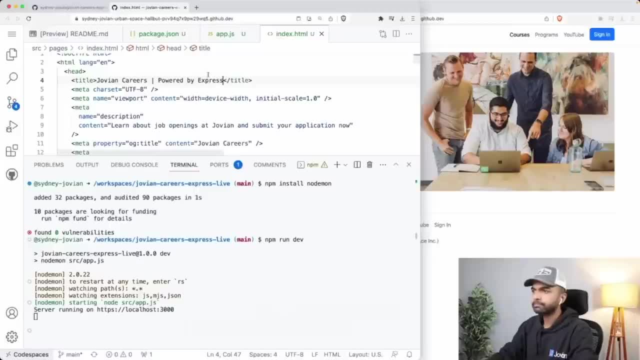 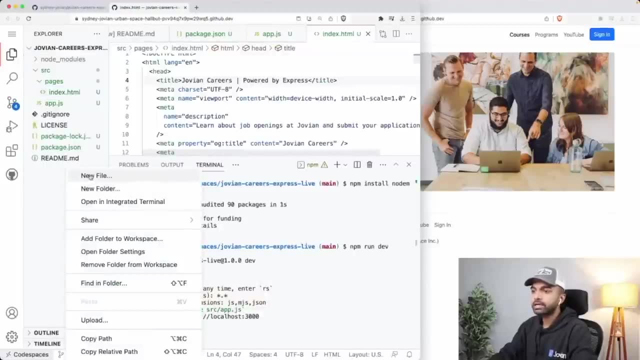 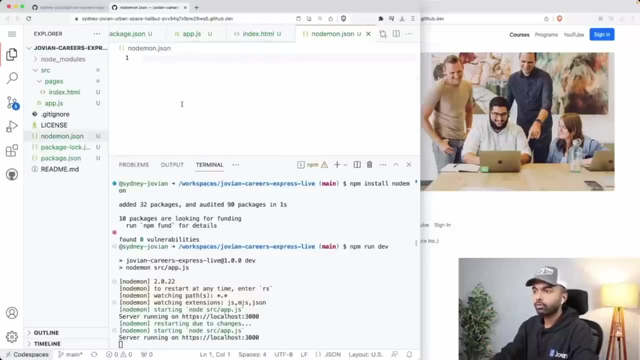 You can see that the server will restart automatically. Well, it looks like it did not. So that's where you also have to configure what causes the server to restart. So we say node Mon or Jason, node Mon dot Jason. That's a new file we put into the root folder of the project. 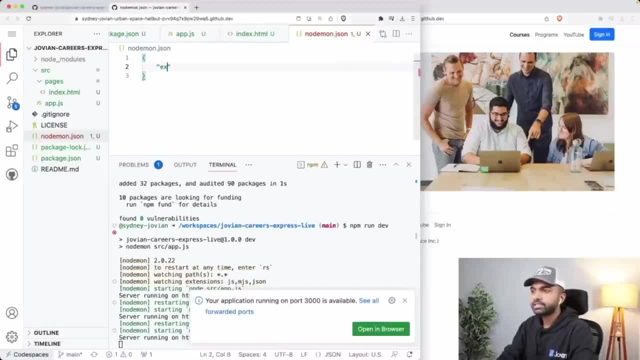 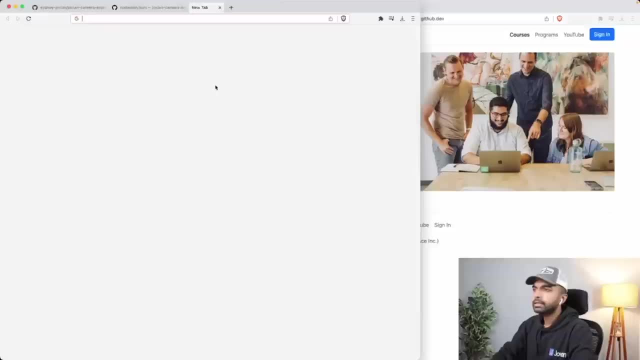 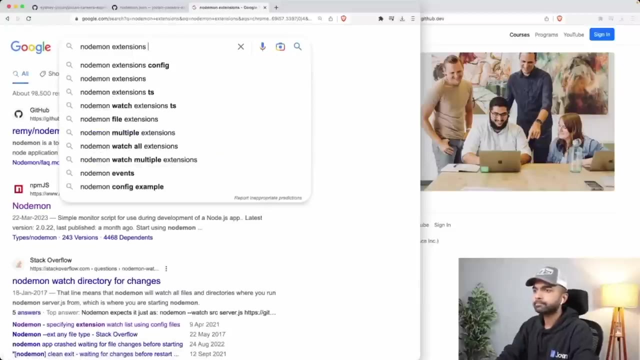 And then we say um, E, X, T, and then we give it the list of extensions for which node Mon should monitor, right? So let's see node Mon extensions, Let's just search that format. Yeah, So you can specify it this way. 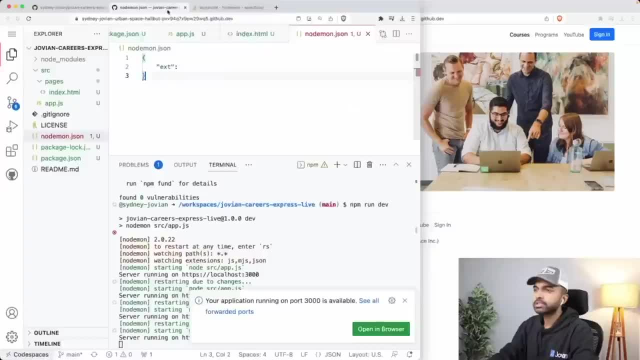 You can say um, E, X, T, and then you provide a list of extensions. So I'm just going to provide a list of extensions here I'm going to. I'm going to say that anytime a JS file or JavaScript file changes, restart the. 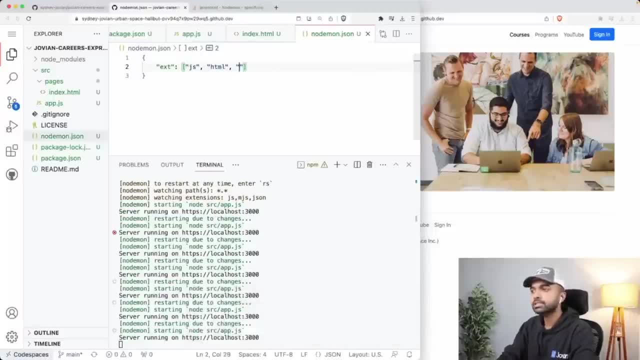 server. anytime an HTML file changes, restart the server. Anytime a styles or a CSS files file changes, restart the server. Anytime a PNG or a JPG file changes, restart the server. So anytime any of these files change, I want to restart the server and let me. 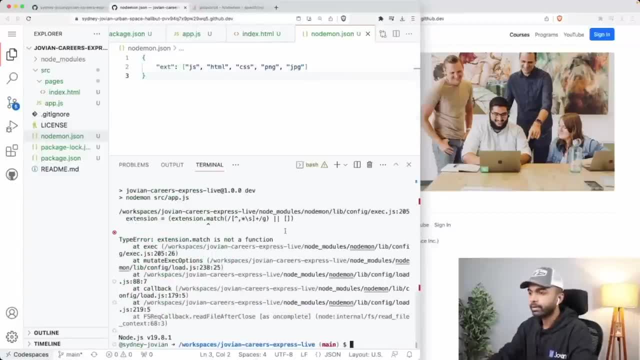 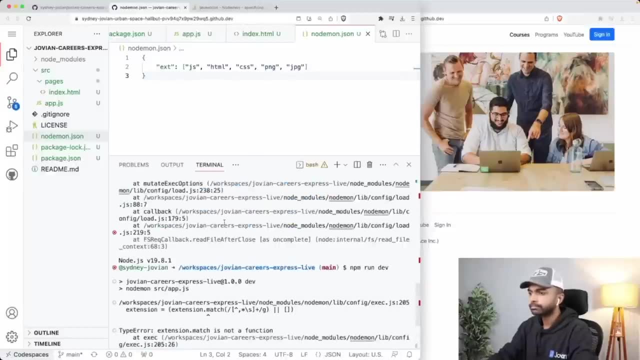 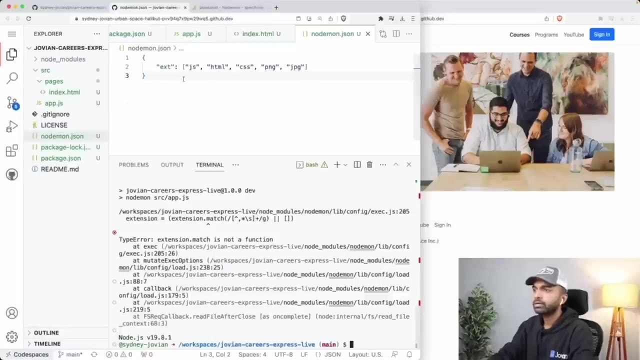 just restart node Mon itself once again. Let's see. Okay, I think I might've missed something up here. Oh, I believe it's just. uh, you do not need it to be an array. Yeah, You just need it like that. 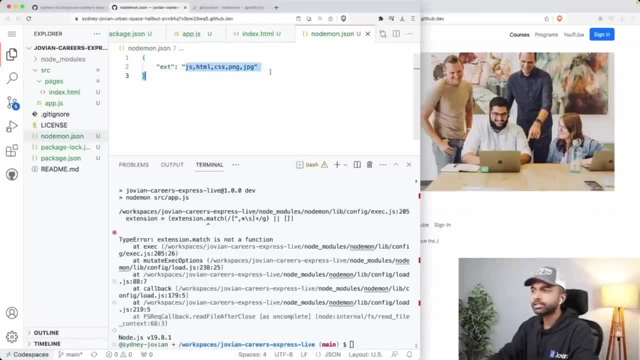 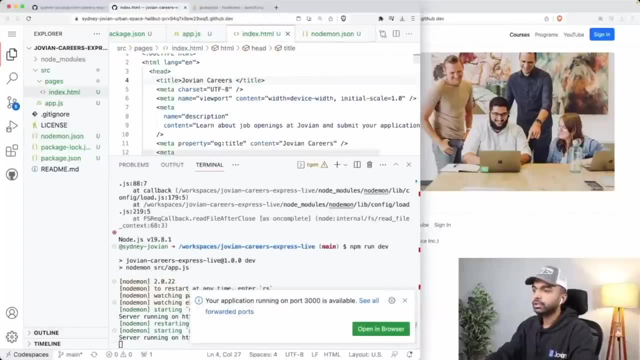 Okay, So you provide a list of extensions as a comma separated string and let's now run NPM, run dev once again, And now you will notice that, Yeah, Anytime we change any HTML file, CSS file, JavaScript file, it's going to restart the server. 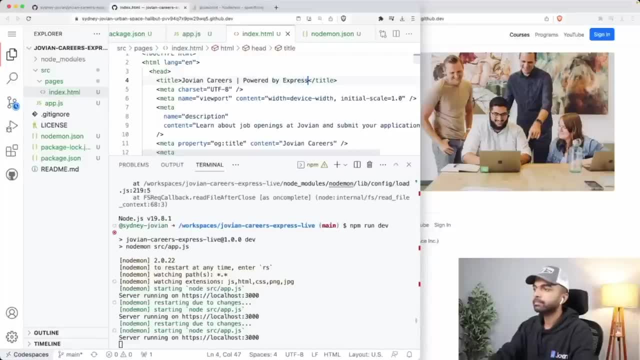 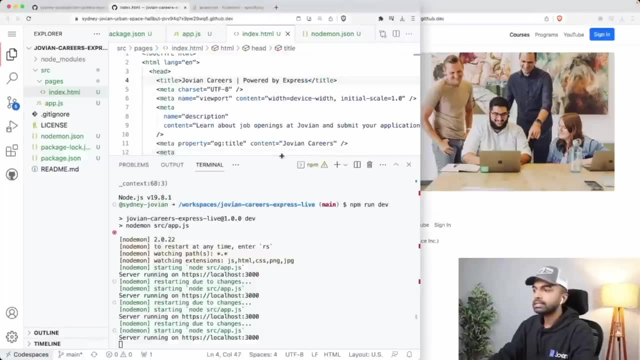 Okay, So I'm just going to say powered by express here and I'll just reload the page. and now you see, here it says powered by express. All right, So that is the benefit of uh, using node Mon. It's going to automatically restart the server, but you still do have to go to 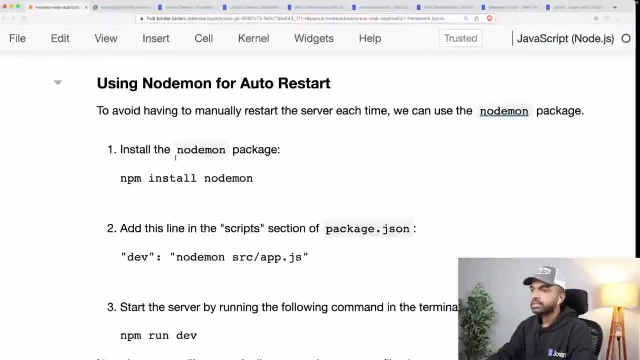 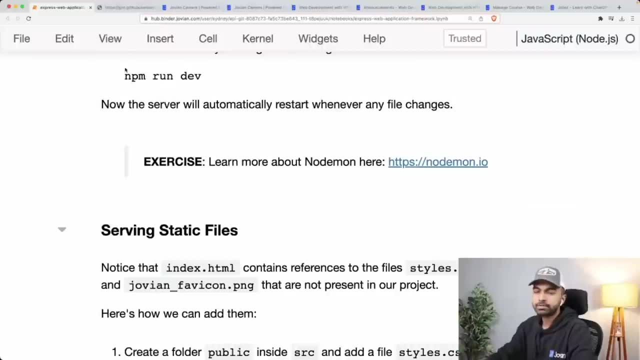 the browser and re reload the page. All right? Um, so now we've set up node node Mon and we are using NPM run dev for development, And when we want to do a Final testing or deployment, then we can just use NPM start. 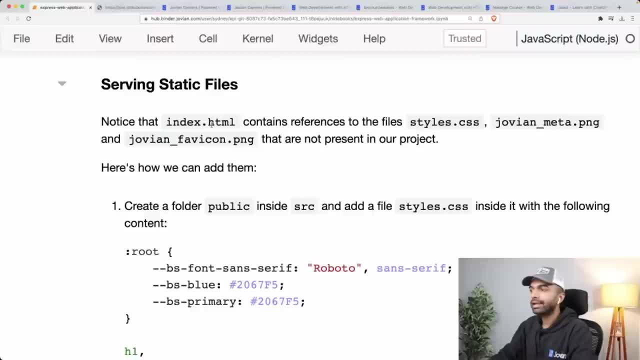 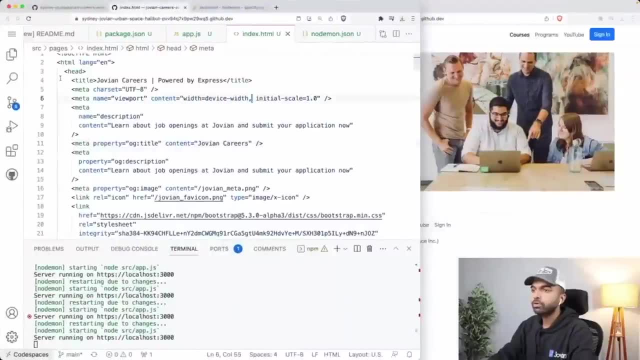 Okay Now the next thing I want to point out is that index or HTML contains references to files like styles dot CSS, Jovian meta dot PNG and Jovian favicon dot PNG, But so far we have not added any of these. 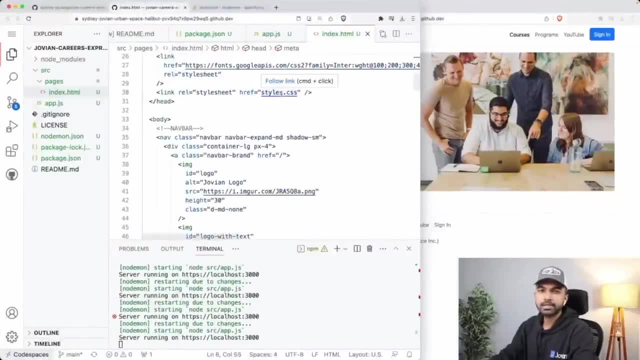 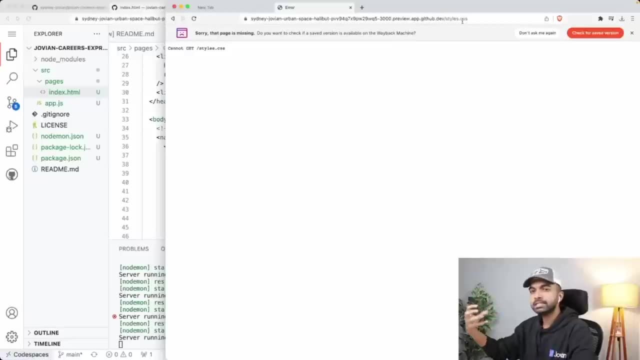 So, uh, you see we are referring to styles or CSS, but there's no styles or CSS file here And, more importantly, there will. there is no styles or CSS file here, So all of these things are executed on the browser. 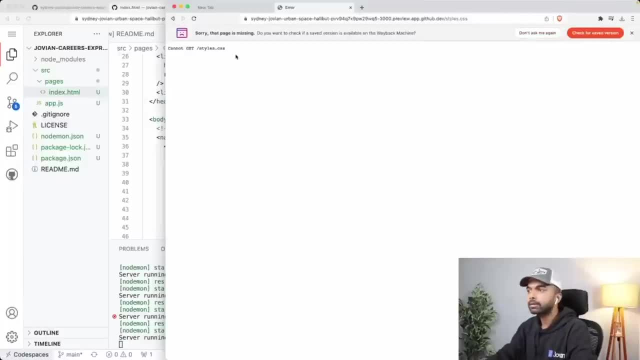 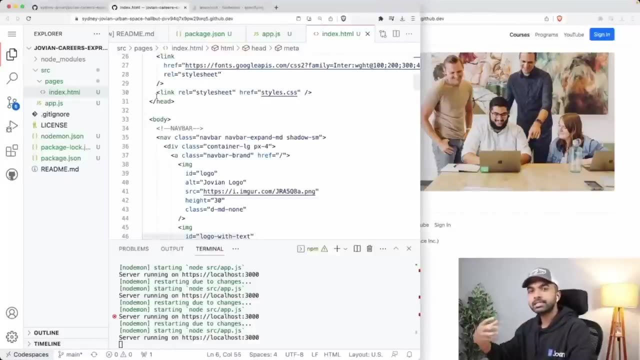 All the HTML is run on the browser And when the browser, when the browser tries to get styles or CSS, it's going to run into an error. So we need to find a way to pass all of these files, styles or CSS, and PNG. 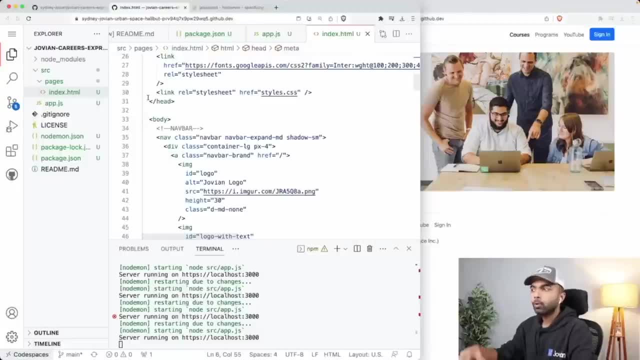 and all of these directly as is, without any changes to our um browser, And that is where we are going to create a folder called static. Okay, So we are going to create a folder called- let me just rename it- public Actually. 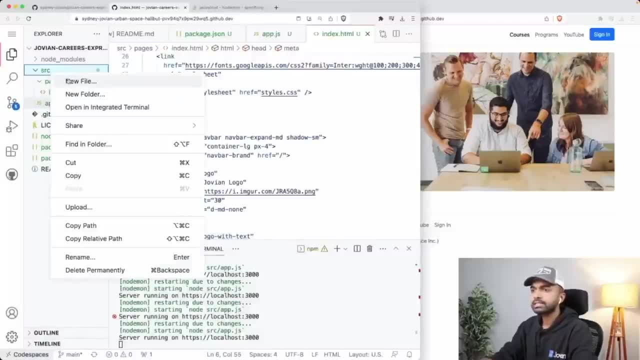 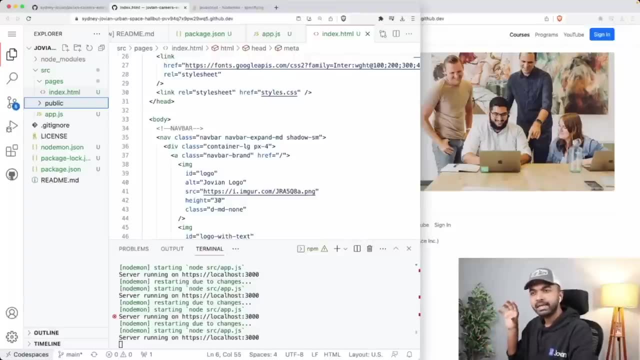 Yeah, Let's create a folder called public, So SRC, public, And into this I'm going to put in all the files that are going to be sent as is, without any change to the browser. Okay, And inside the public folder let me put, for example, styles, dot, CSS, and into. 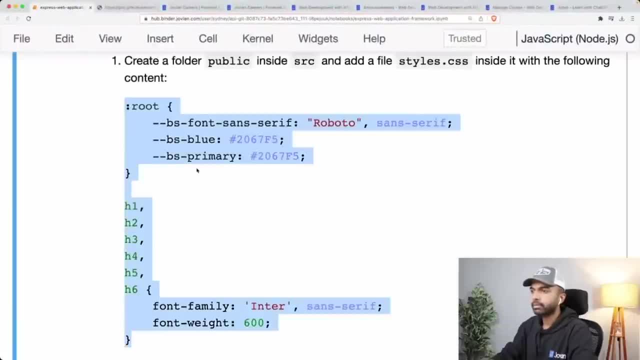 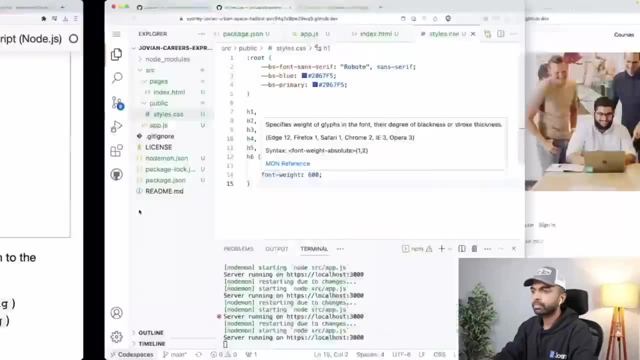 the styles or CSS. let me put in some content. All right, Okay, I've put in some content into styles or CSS. It looks like I have one more piece here. Yeah, So all we're doing in the styles or CSS is maybe. 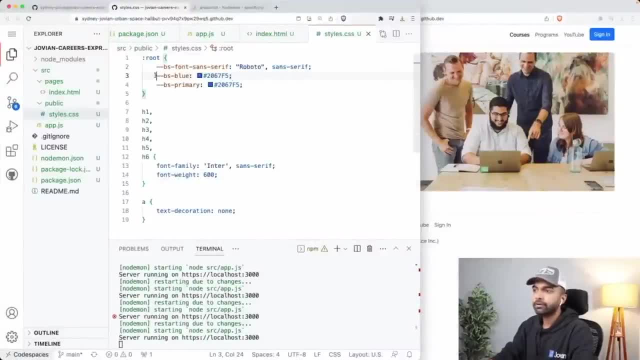 Configuring the default font, body font and configuring, configuring the default blue color and the primary um color on bootstrap. So these are all CSS variables we're configuring. And then we are also configuring the font family for the heading. So we are using the inter font family which we have included within our index. 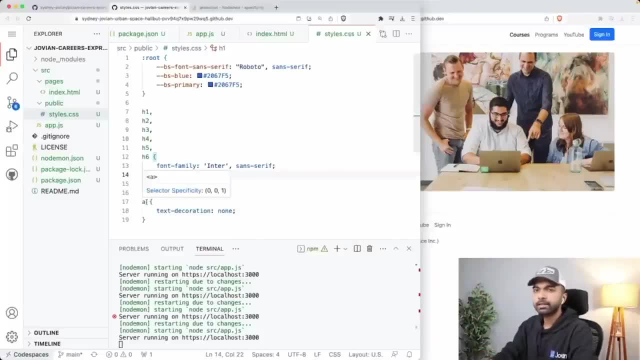 or HTML page from Google fonts, And we are also configuring that the eight tags or the link tags should not have any underline. So text decoration underline is the default. We are setting it to text decoration or none. Okay, So that's a styles dot CSS file. 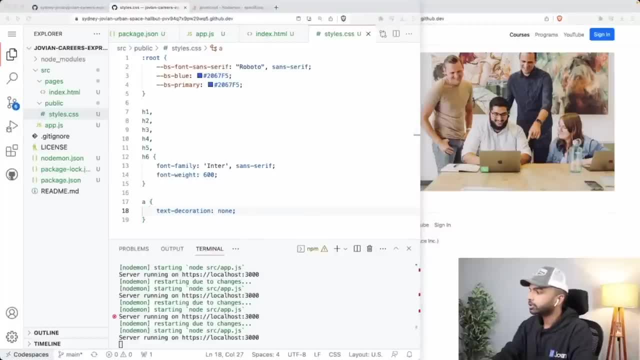 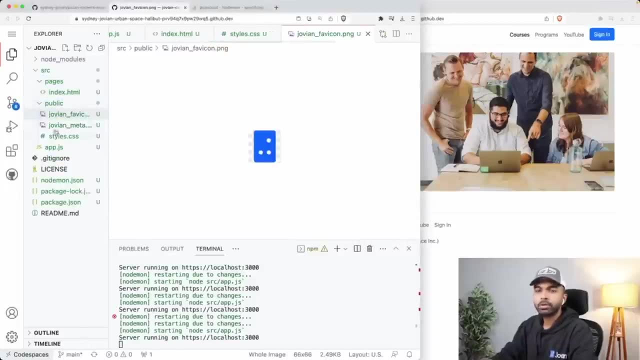 Next, I have a couple of these files. I have this file, uh, Jovian favicon dot PNG and Jovian meta dot PNG on my computer. I'm going to drag them in here and put them both into this public folder as well. 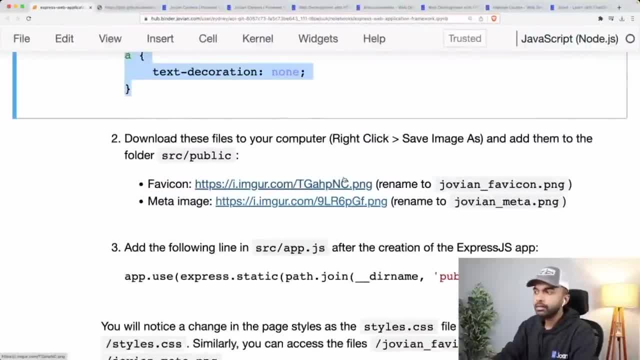 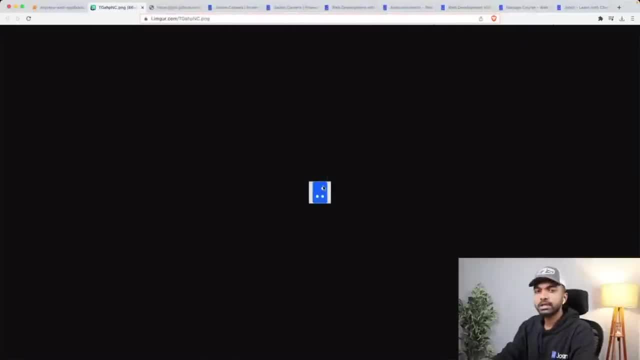 And you can download these files from these URLs. So just go into this URL and right click and save it as Jovian favicon dot PNG and Jovian meta dot PNG. So this is what the Jovian favicon dot PNG looks like. 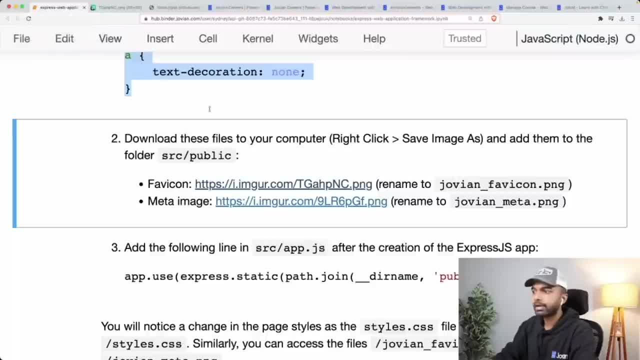 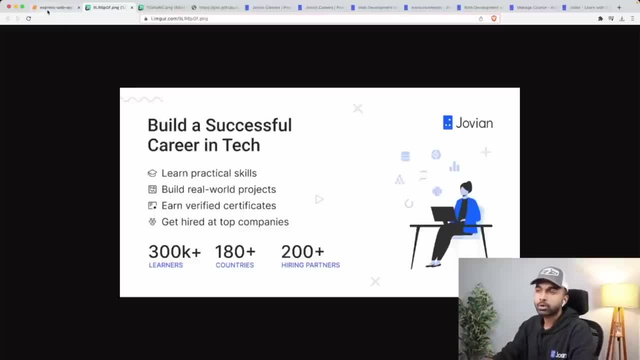 It is going to be used to configure the favicon or the icon in the browser, And this is what the Jovian meta image looks like. This is simply going to show up when we share that link with somebody else on show on social media, et cetera. 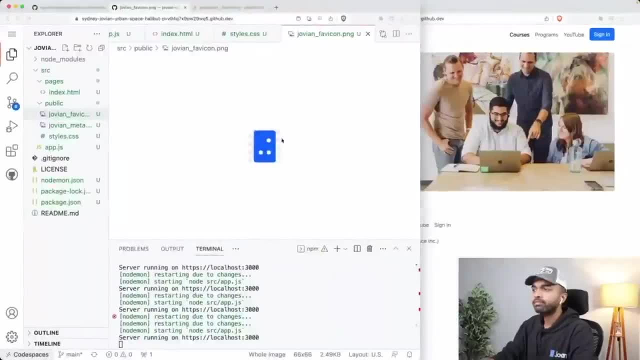 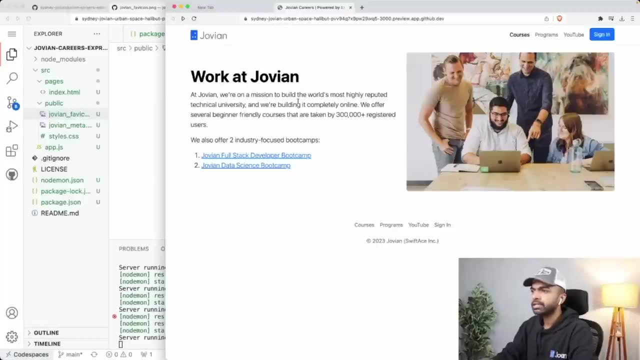 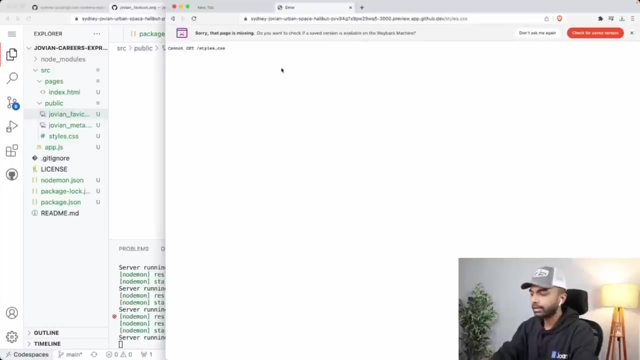 Okay, So, um, all right. So now we've added these files: styles dot, CSS, index or HTML. uh uh, styles or CSS, Jovian favicon, Jovian meta- but nothing seems to have changed. Even if I try to access slash styles dot CSS, I still cannot get it. 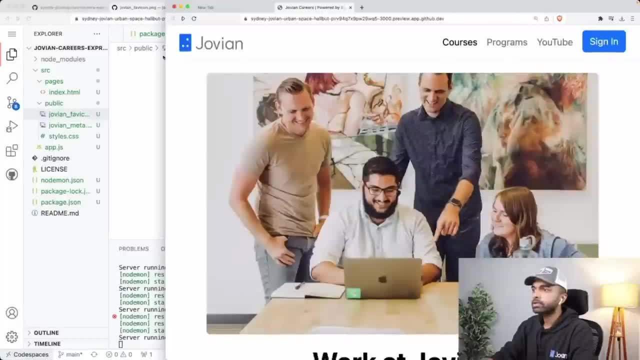 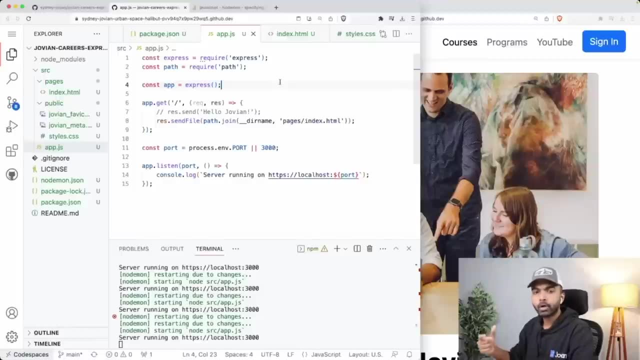 So it's still says: cannot get styles dot CSS. So what do we do? Well, you actually have to inform, express that there is a certain folder on your, in your project, from where you want to directly send all the files to the browser. 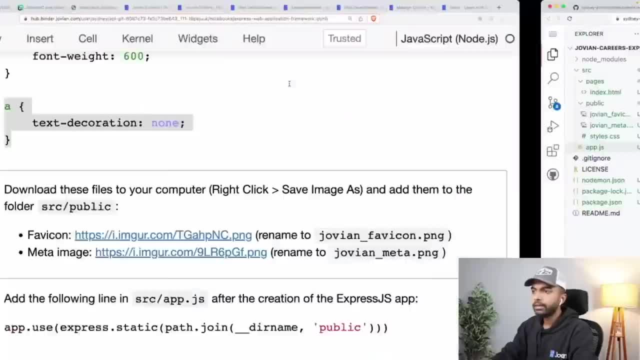 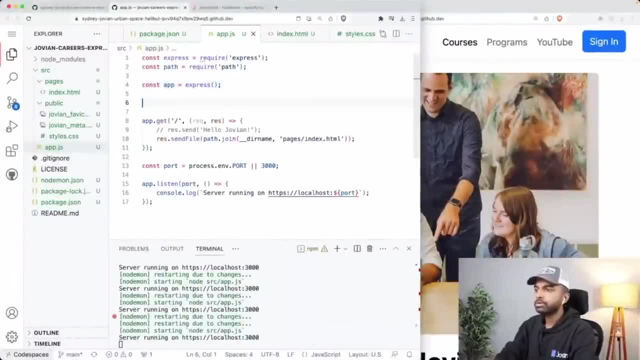 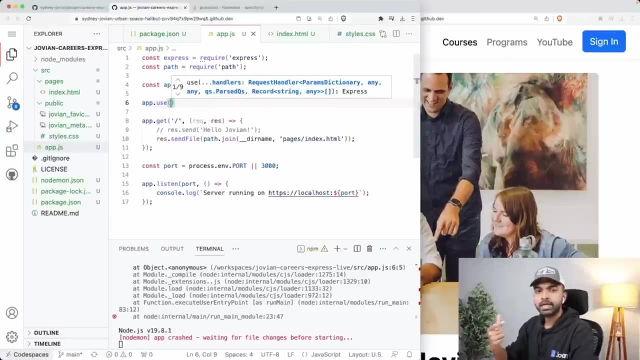 You don't want to make any changes to them. Okay, So how do we do that? The way to do that is by just adding this one line within express. So we say app dot use. after creating the app, we say app dot use. and app dot use is a very common pattern in express, where any new feature 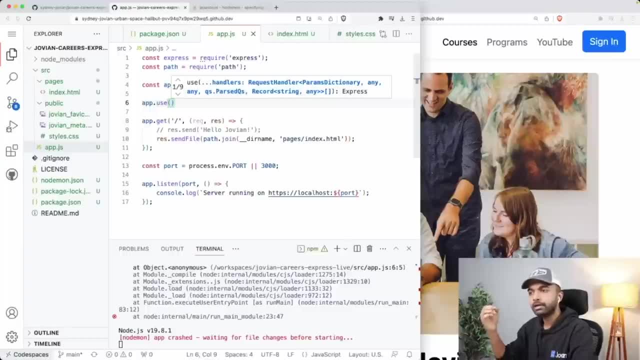 You want to add any what's called middleware in express, any new features you want to add, you just add them using app dot use. And here in app dot use, we are going to use: uh, we're going to set up a static folder using express dot static and we need to give it the exact directory name. 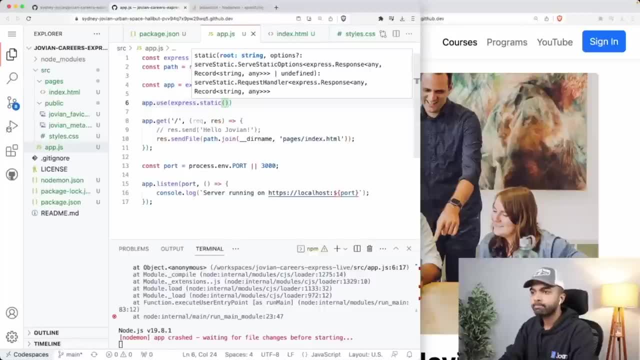 So all the four, or the full path of the directory where this, um, all these static files are located. Okay, So I'm going to say path dot, join, underscore, underscore, DIR name, which is simply getting the name of the current directory, Slash. 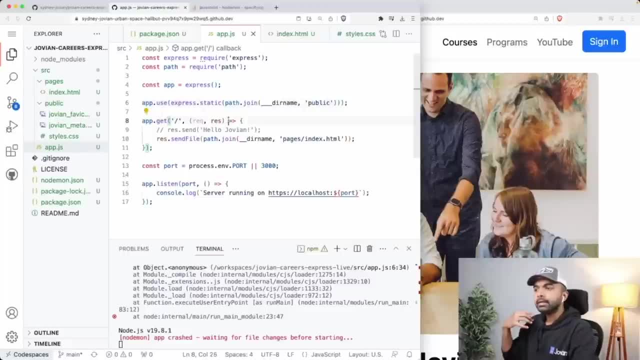 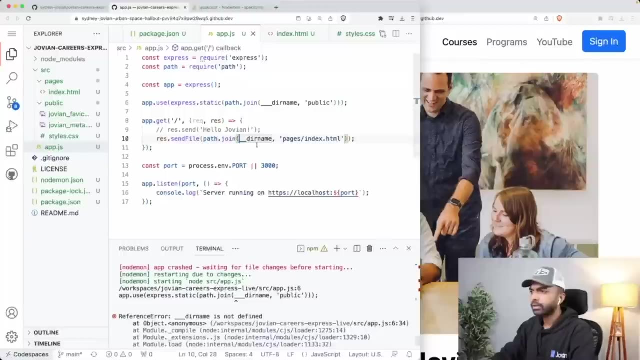 Public. So what we're saying here is: take everything that is there in this folder called public and send it to the browser as is when requested. Okay, And now it says the app crashed. Okay, I put in an extra underscore. So yeah, now the app should have restarted. 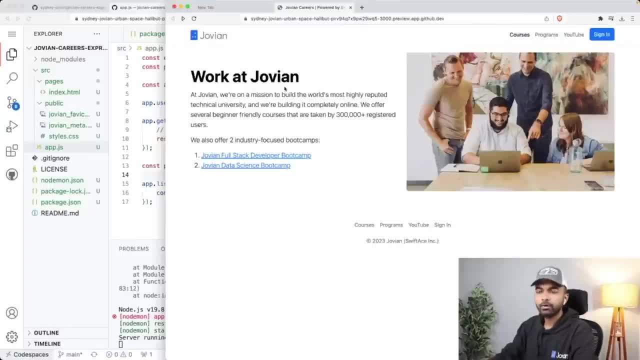 Yep. So now the app is restarted And now, if I reload the page, watch closely, you will notice the fonts change. There you go, You see The fonts just changed and you can actually see here. If I open slash styles dot CSS, you can see that now we have this styles file. that is served. 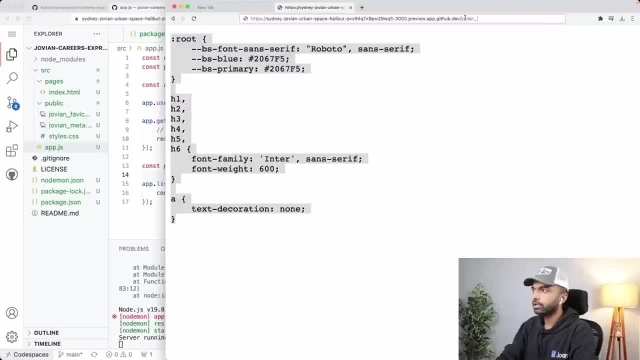 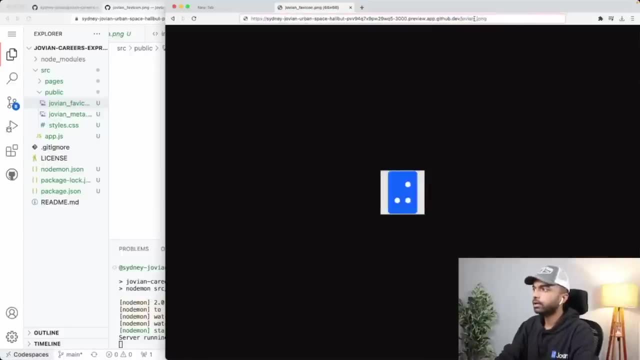 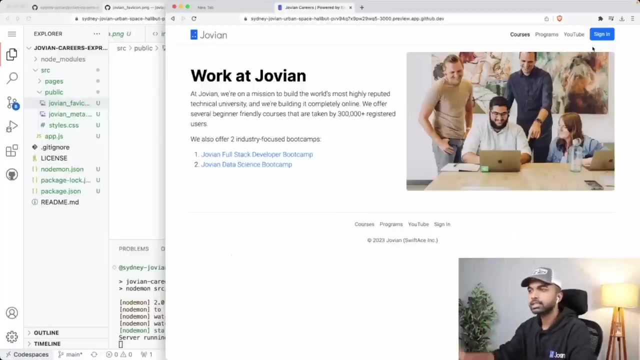 And if I open slash Jovian underscore favicon dot PNG, you can see now the favicon is getting rendered. If I open Jovian underscore meta dot PNG, you can see that our meta meta image is getting rendered as well. Okay, And all of these are linked from index to HTML as well. 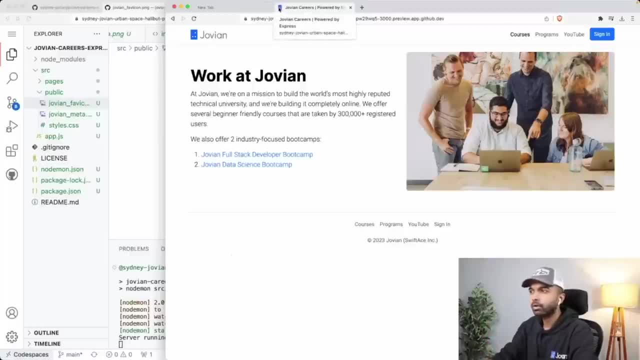 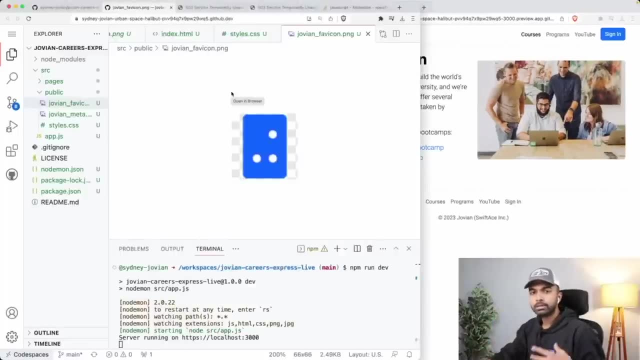 So that will show up properly too. You can see here, it shows the nice icon here in the browser tab. So that's one other thing. I want you to take away anything that you want to directly send out to the, uh, to the browser. 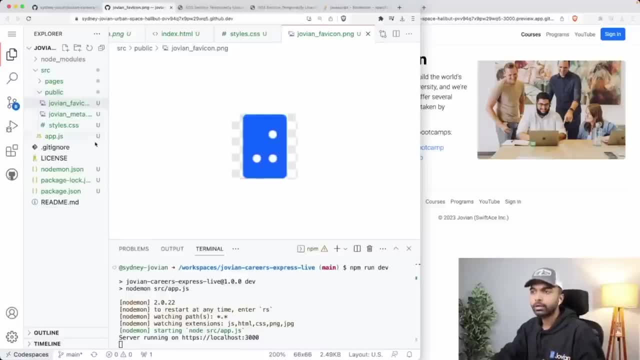 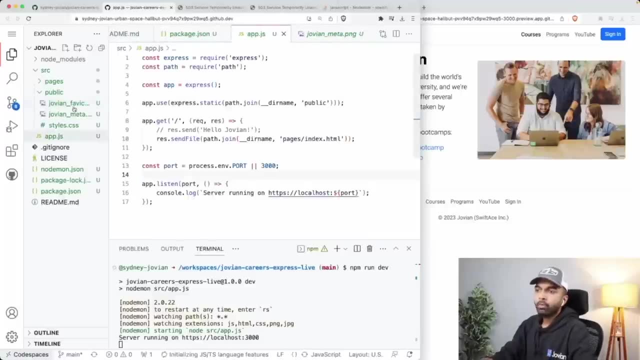 Then you simply create a folder and put all of those files into a folder and you simply configure a static folder within app dot use. Okay, Now, we didn't do this for index or HTML, because we're going to make some changes to index or HTML. show some dynamic data on that page. 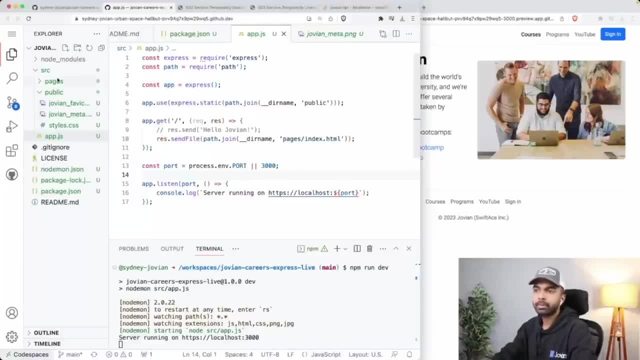 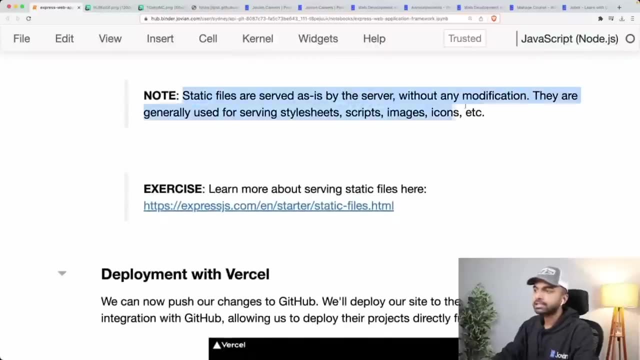 That is why we want to process it before we send it. That is why we didn't put it in. That is why we want to process it before we send it to the public or static folder. Okay, All right, So just keep that in mind. static files are served, as is, by the server, and it is generally used for style sheets, scripts, images, icons that you just want to pass on to the browser directly. 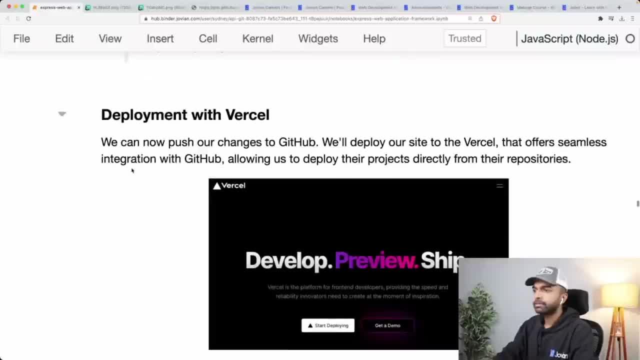 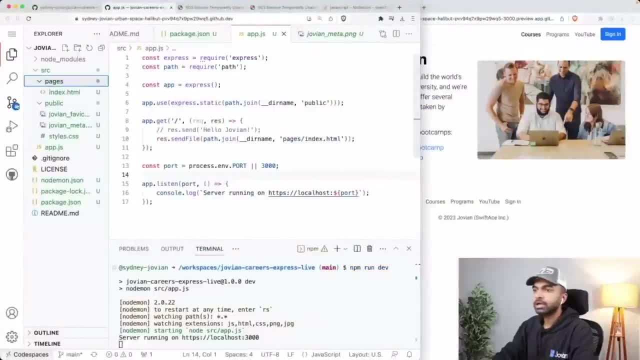 And you can check out this resource to learn more about static file serving. Now one last thing we can do is to simply push our changes back to GitHub and then deploy it to Vercel. So I'm just going to come in here into the git. 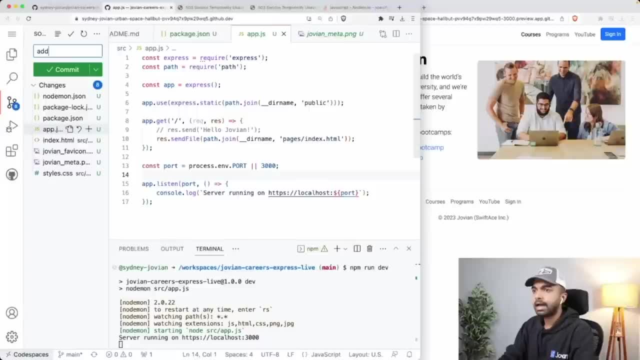 Tab of the server, Okay, Of the sidebar, And I'm just going to say I did basic. uh. well, added express app index, dot HTML and static files. I'm going to click commit and that is going to simply stage and commit all the changes. 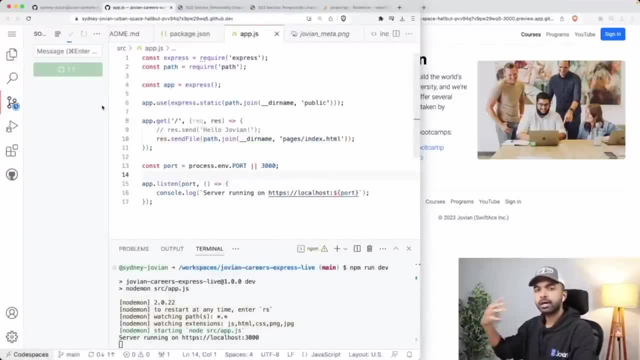 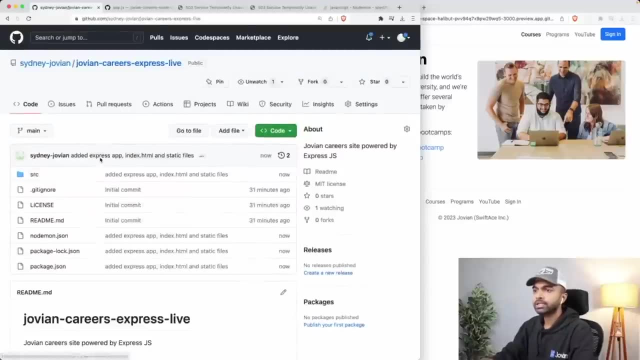 And I'm going to sync this back to GitHub. So stage commit and sync, three-step process And once this is done we can go in here and you can just reload this page and you can see here that we have this SRC folder, We have this package or JSON. 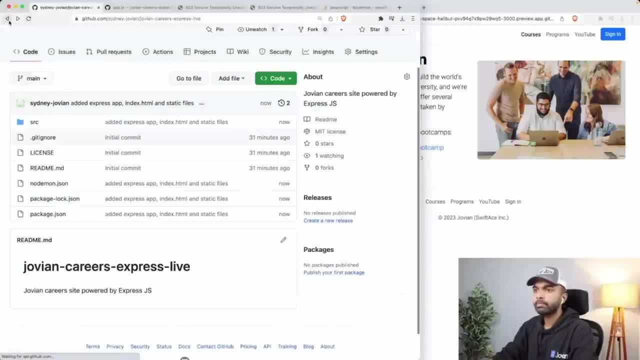 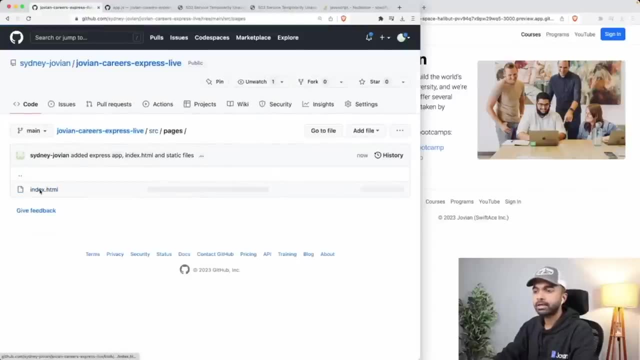 You can see package or JSON has the dependencies express and node mon and there's no node modules folder because it is ignored in the git ignore in the SRC folder. has a pages folder where it has indexed or HTML. Of course it has app and it has this styles or CSS et cetera as well. 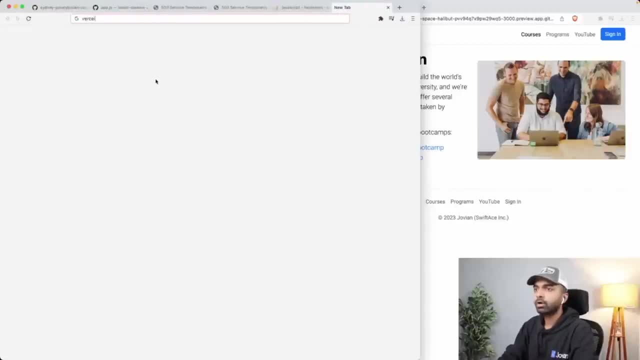 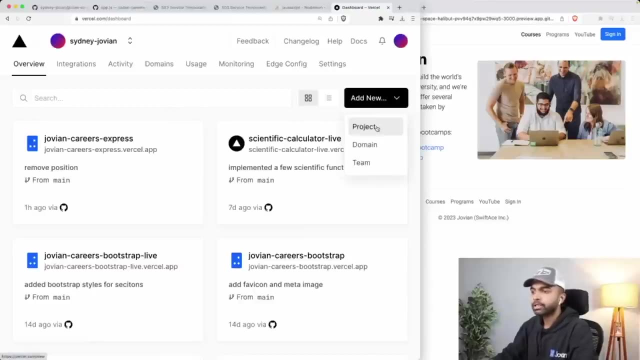 Okay, Now let's deploy this. So I'm just going to go to Vercelcom, and Vercel is the platform we typically use for deployment, because it's really easy to use. That's what jovincom is replied on as well. 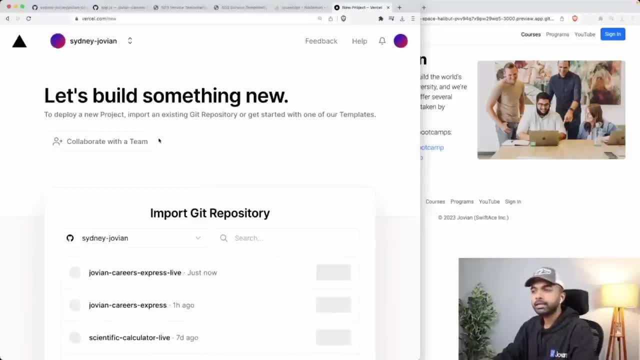 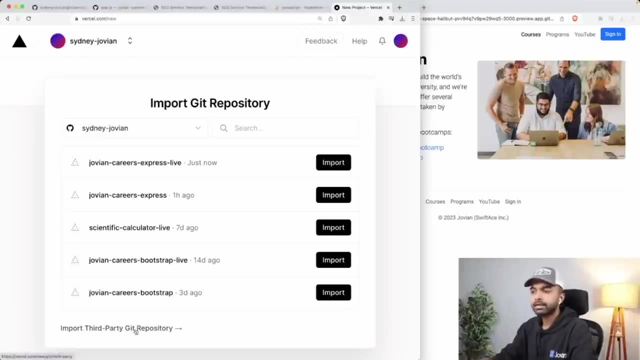 And I'm going to select Add new project here. And if you haven't connected your GitHub account, you can connect it here If you can. if you haven't connected all the repositories, you can configure your GitHub setting here as well. 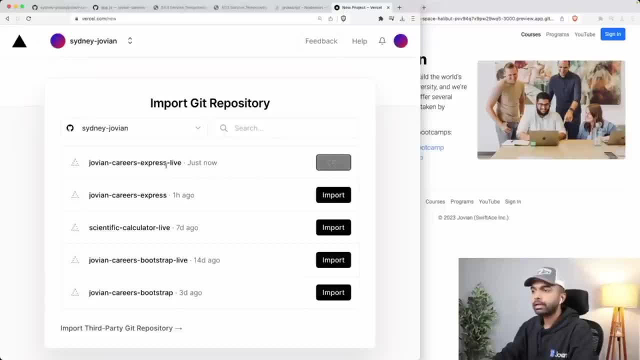 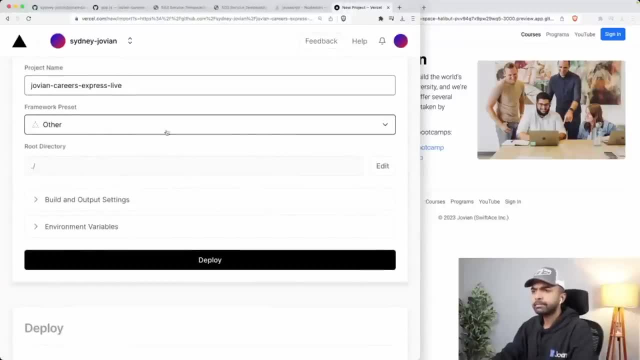 But in this case we're simply going to go into the Sydney Jovian account and import Jovian careers express live, And when we import it, we can select the framework preset. Okay, Now, there's no framework preset here And because this is just express, there's no framework as such. 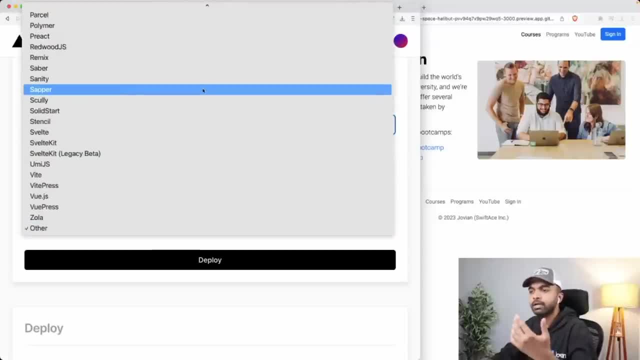 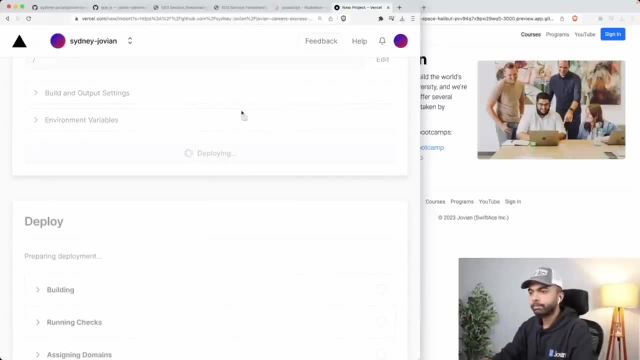 It's just a. In fact, Vercel does not have inbuilt support for express, but the root directory is just the directory which contains the package or JSON file And we can click deploy. Now, hopefully, what they should do is they should look into the package or JSON file and it should deploy. 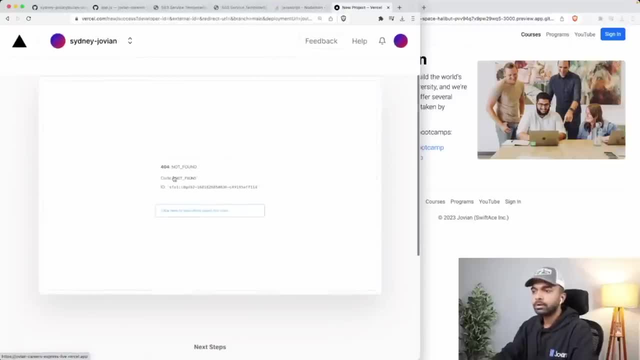 And let's see if that happens. Okay, So it looks like the deployment is complete, but if we try to access it it says 404 not found, And this is because Vercel needs things to be configured in a certain way. 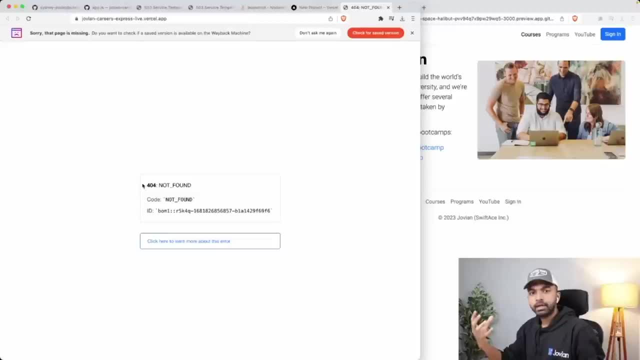 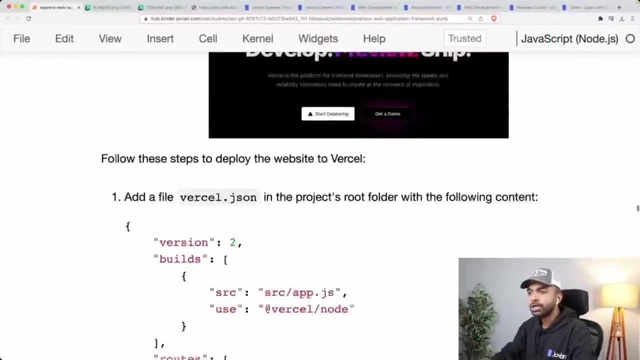 Vercel needs to be told what is the root file that we need to access. Vercel needs to be told what are the different ways in which different routes need to be handled. So there is one special piece of code that you need to add when you're deploying an express application to Vercel. 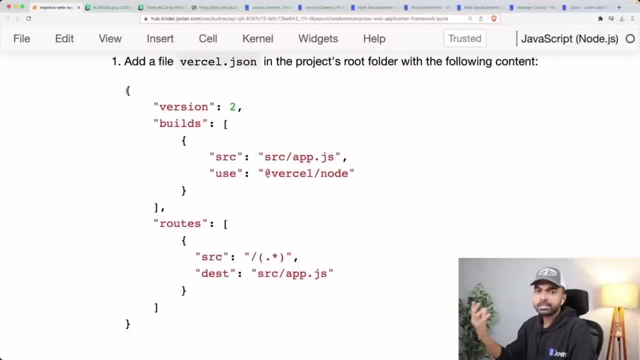 Okay, And again, this is not something that you know by default. this is just something that you would normally Google and figure out, but you need to add a file called Verceljson that informs Vercel a few things. 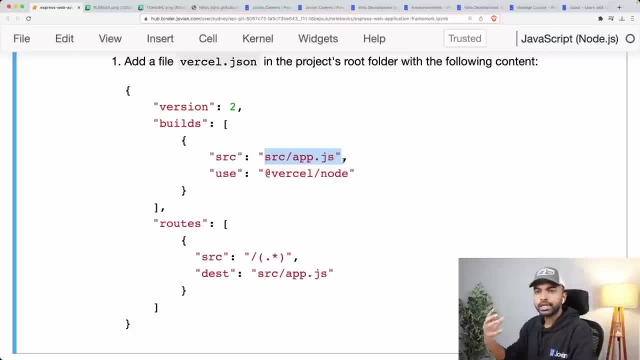 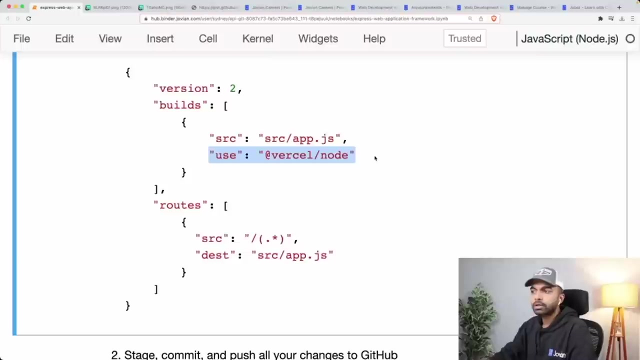 One. It tells Vercel that SRC is limited. It tells Vercel that SRC is limited, Exactly. Uh, so let's establish this, Let's initialize this And we're going to give a number of brackets and, no matter what route we try to access, we want them all to be sent to appjs and we want. 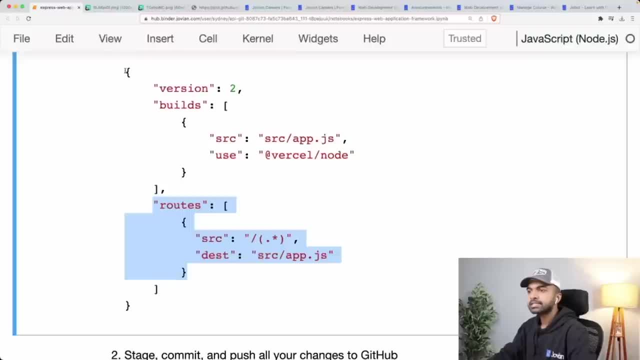 appjs to handle the routing and not Vercel itself. So that is again something that is configured. And again, don't worry if this seems confusing: whenever you are deploying an express JS application to Vercel, you simply copy paste this or find it online. Okay, So let's go back. 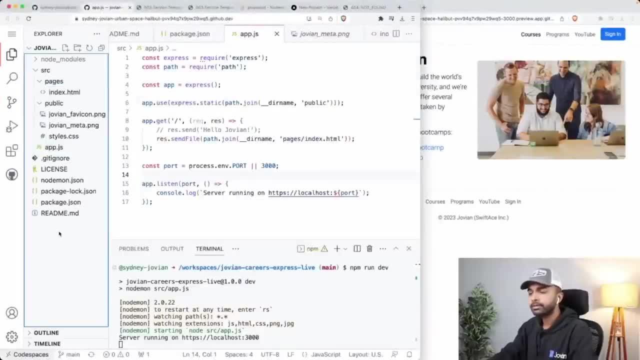 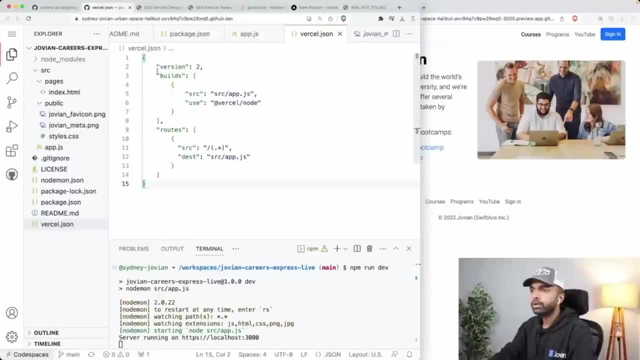 here and let me go in here and create a Verceljson file. So new file, Verceljson. And in this file I'm just going to put in this code version two builds routes, just standard code for configuring Vercel to run with express And I'm just going to say: add Verceljson. 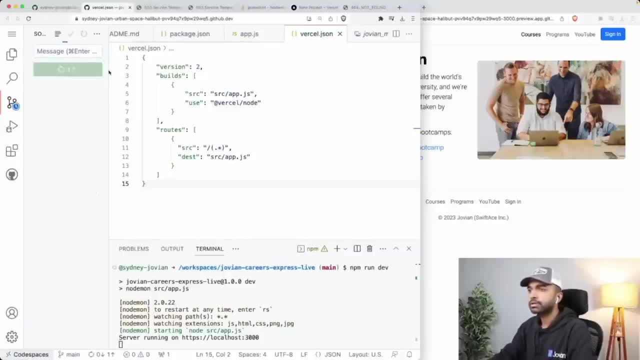 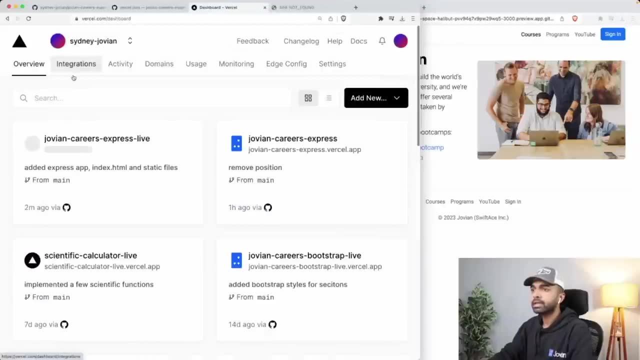 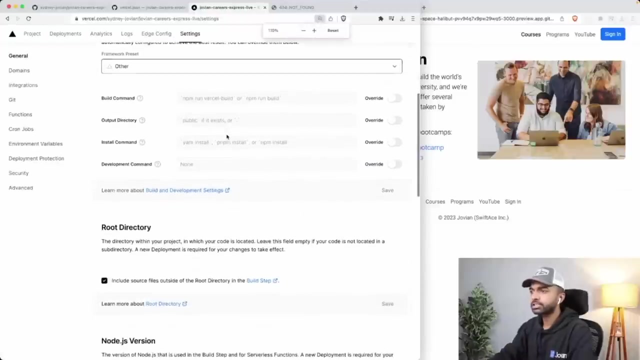 And let me click commit and sync it And that should now get sent up to the server. And now let us go back into our Vercel dashboard. Let's go back into Jovian careers express, live, and delete this project and just create a new one with the Verceljson file. 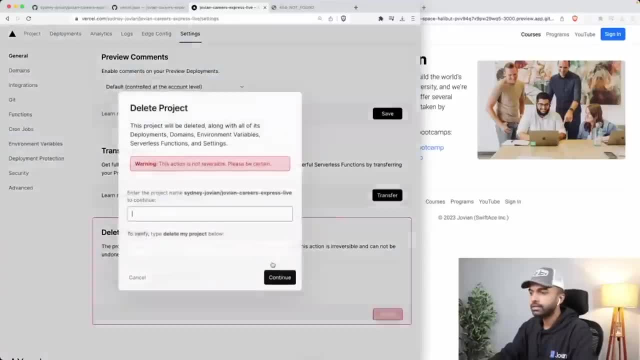 So sometimes what happens is, if you change the Verceljson file, you may have to just recreate the project. So I'm just going to delete this project And you can delete the project from the project settings. And let's check the Verceljson file. So the Verceljson file looks. 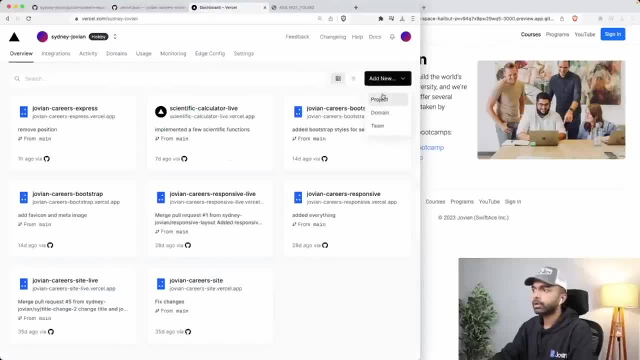 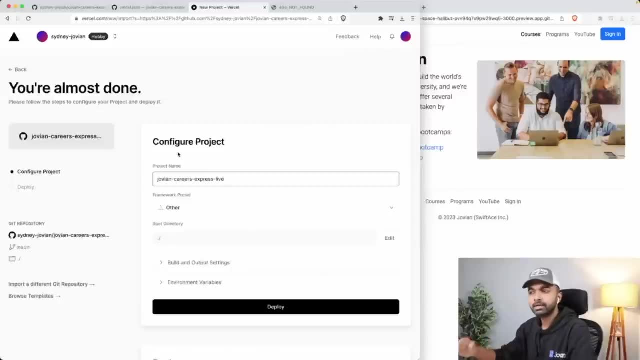 fine to me. And now let's come back into Vercel and create a new project. So now once again I'm going into new project and said I'm selecting the Jovian careers express live project which has the Verceljson file already No framework preset. 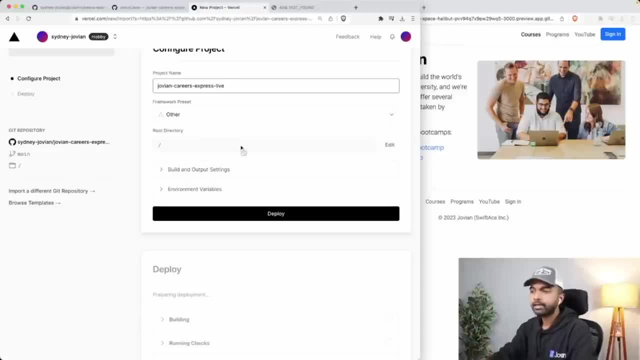 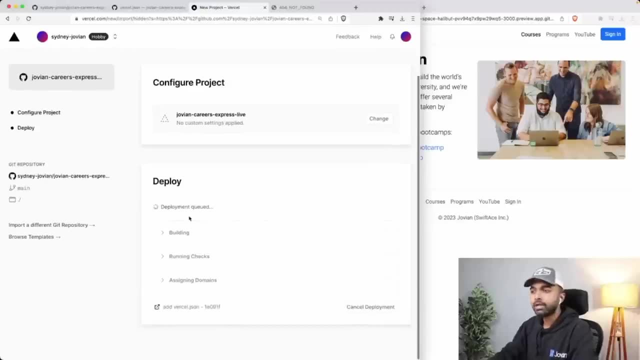 And the root directory is just the dot slash which is the root of the entire directory, because that's where the packagejson and other files are present And I'm just going to click deploy. Okay, And hopefully this time it should pick up the settings from the Verceljson file. 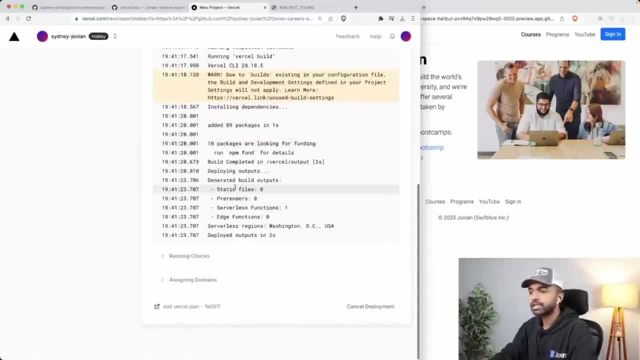 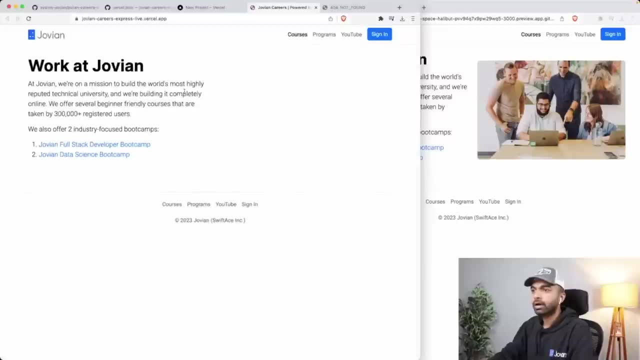 Yeah, looks like you have a Verceljson file, So it's going to pick up the settings properly And let's see if it's going to do that deployment this time And it does, Perfect, So our application, or our web web server, is now deployed. 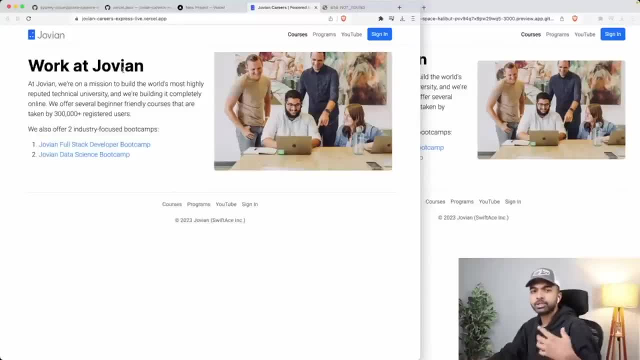 To Vercel And it is now scalable. So our code space machine can shut down anytime And it cannot scale. but Vercel will automatically scale things depending on the traffic And it will automatically redeploy whenever you push to the main branch. So that's it. So now we have a basic deployment. 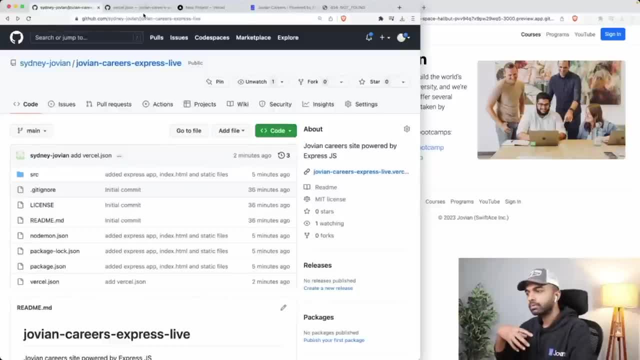 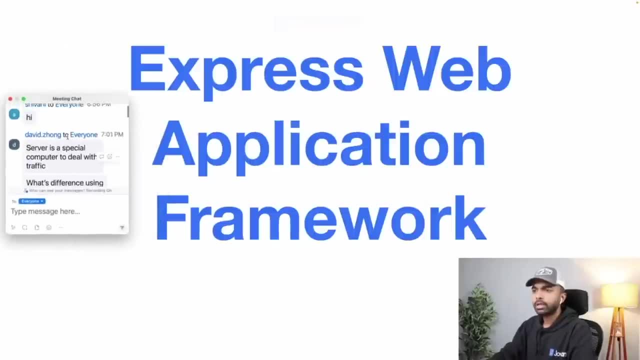 ready as well, And now we're ready to start maybe rendering some data dynamically into that page. Maybe let's see if we have any questions at this point already. Okay, there's a comment here. server is a special computer to deal with traffic. That's right. Yep, that's right. 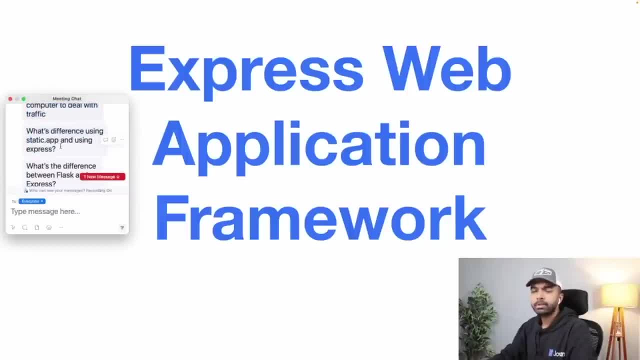 That's a good way to look at it. What's the difference between using static dot app and using Express? So, starting that app, all it does is it takes the files that you have and it gives them to the browser when requested. In Express we can write some custom logic, for example: 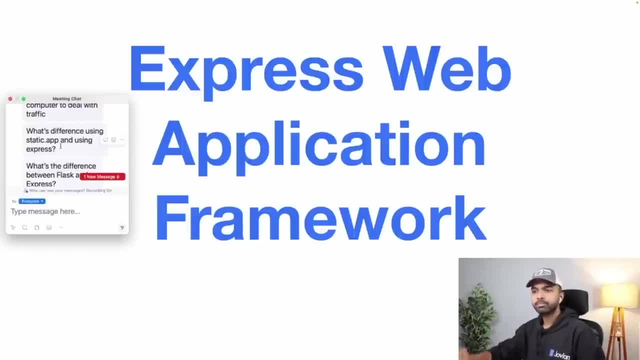 fetching data from a database, sending an email, handling form, submissions and all of that. Okay, so I hope that answers that. What is the difference between Flask and Express? Well, Flask is a Python web framework. Express is a JavaScript web framework. they do the same thing. 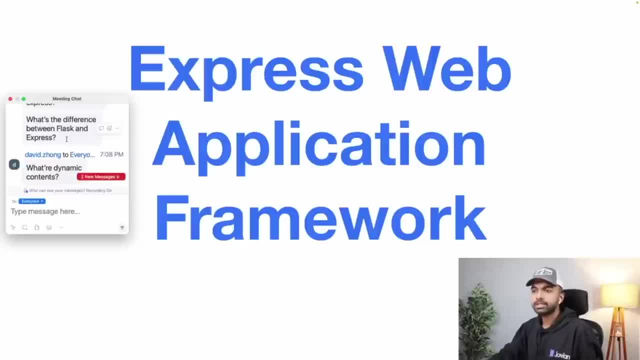 they are both the smallest possible frameworks, essentially in each of those languages, But that's basically it. What are dynamic contents? So anything, any data that is, for example, fetched from a database. for example, if you go to my Jovian profile. 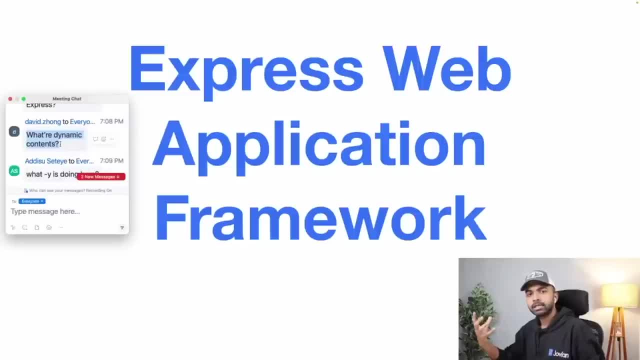 each time you open it you'll see something different, because I may have worked on new notebooks in the meantime. Now, obviously, I'm not creating an indexhtml file and putting it up each time I create a new notebook. this data is going to be fetched from the browser, from a database. 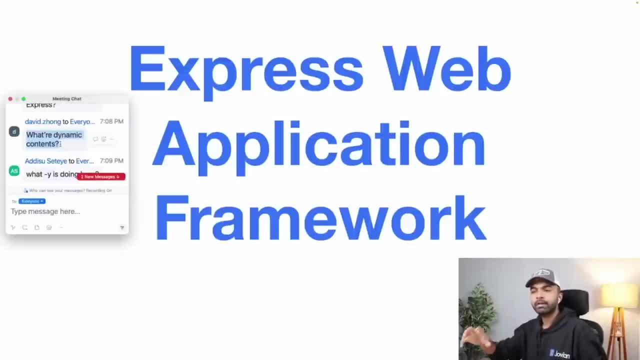 And that HTML file is going to be created on the fly when you try to request it. Okay, what was minus y doing here? So when I said npm init minus y, I will let you search that online. All it does is well, it makes our work. 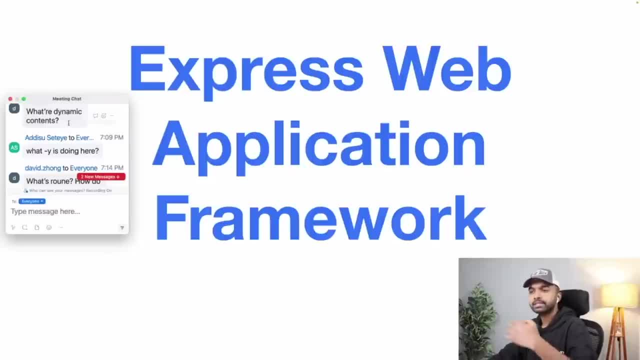 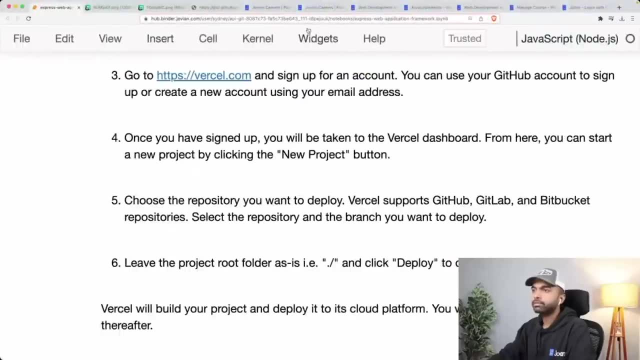 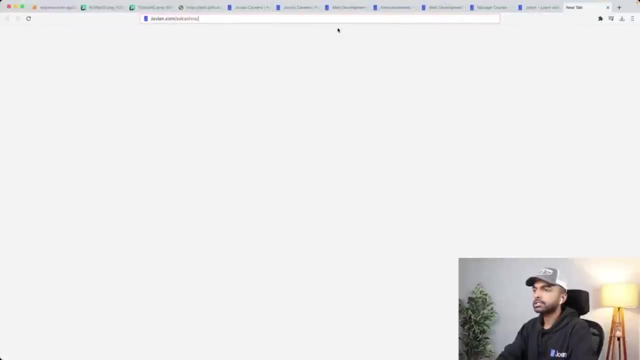 a little easier, Otherwise, npm init is going to ask you for the package name, etc. etc. Okay, what is a route? Well, a route is simply a path on the page. So, for example, if you have, for example, if you have joviancom slash, Akash NS, that's a route right. 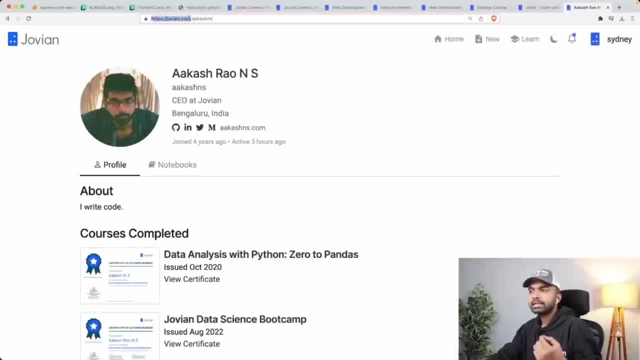 So if you have a route, that's a route right. So if you have a route, that's a route, that's a route. so slash Akash NS, so joviancom, here is the domain and slash Akash NS is the path or the. 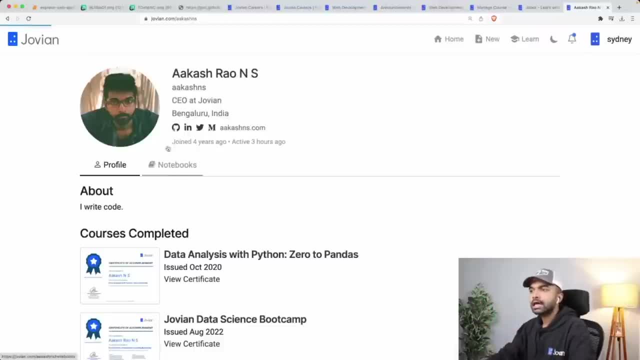 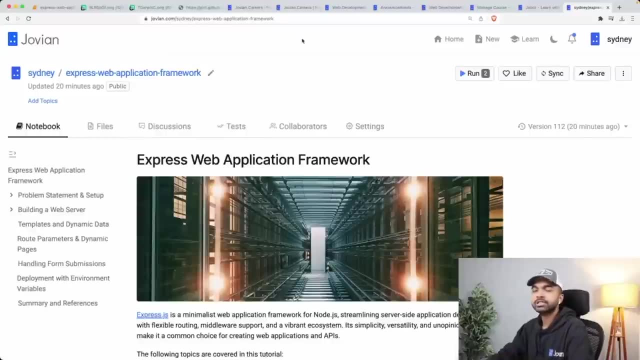 route, which is where, within the server, do you want to go? or slash Akash NS slash notebooks, which is what you see here. that is another route. or slash Akash NS. or slash Sydney slash express web application. that is another route. or slash learn slash courses: that is another. 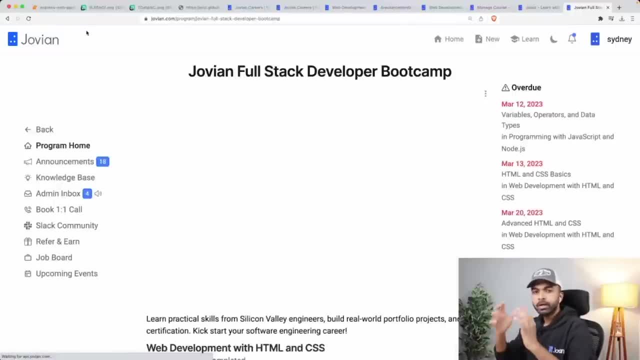 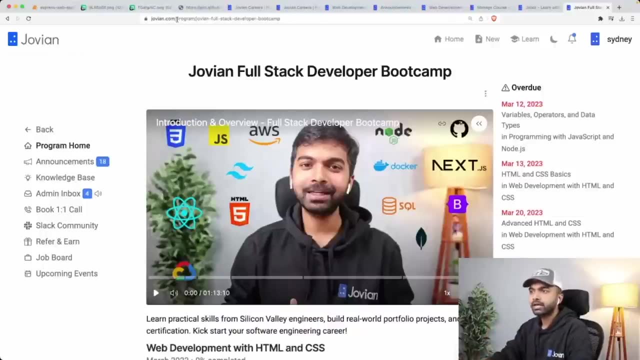 route, or slash, learn, slash full stack developer bootcamp, that's another. So these are all the sub paths that you can have present in your application And we've just looked at the root route, which is where there is no sub path, which is just joviancom or wherever, or in this. 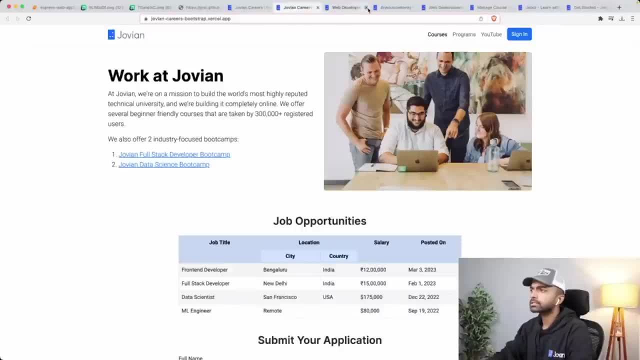 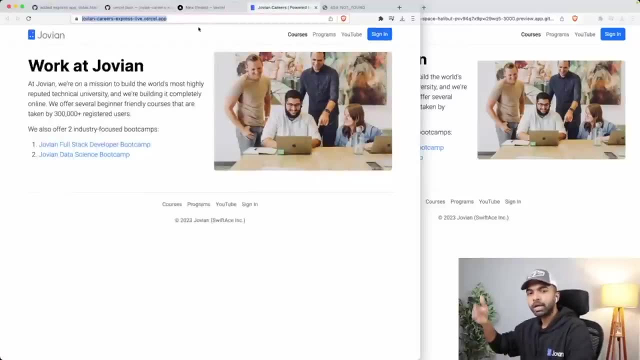 case it is deployed at jovian careers. In this case it is deployed at jovian careers: live dot, Vercel dot app. So that is what we've looked at so far, But we look at some sub routes as well. 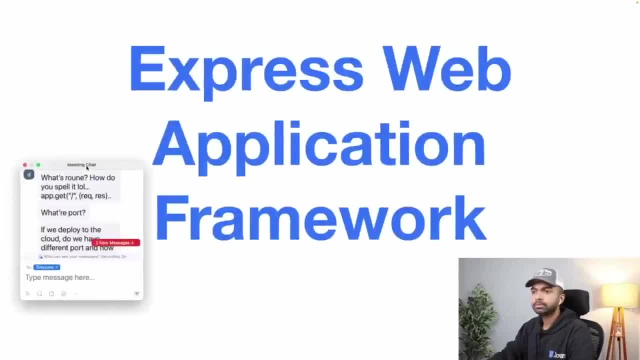 shortly. Okay, what is a port? Well, as I gave the mailbox analogy, let's say in a building you have a bunch of people living and everyone needs to get their mail delivered. So that's where there's a mailbox And the mail for each person comes into the. 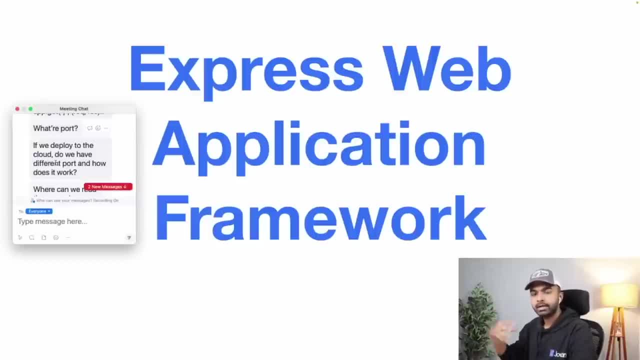 respective mailbox. In the same way when an application is running, when a server is starting on a particular computer- and there are many servers all the time running on your computer- internal processes that you may not be familiar with. each of them can can put their claim on. 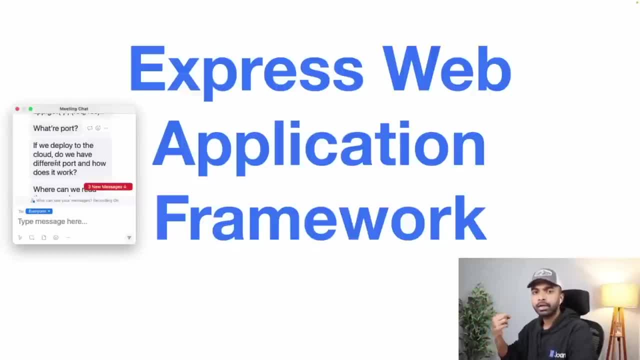 a port and all the requests, messages sent to that port are going to get delivered to that server. So that is something the operating system provides. If we deploy to the cloud, do we have a different port And how does it work? Yeah, So when we deploy, the cloud will deliver something that will. 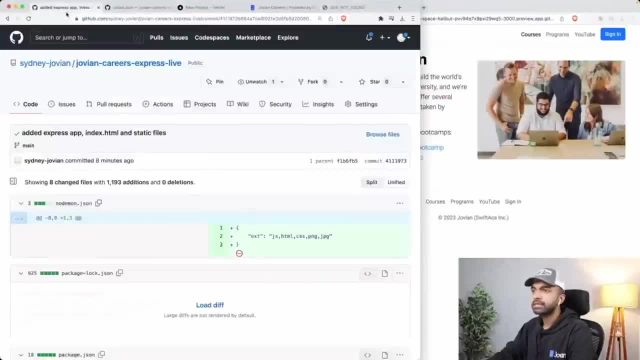 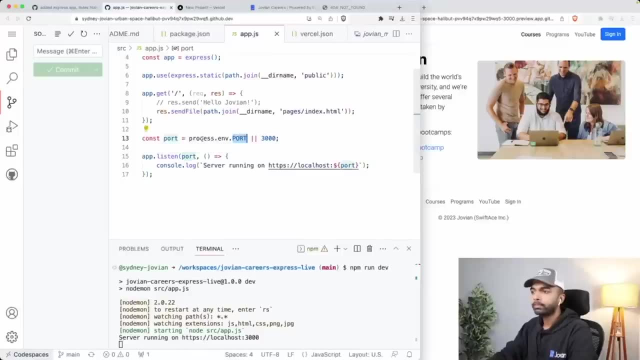 be delivered to the port in one minute. But ideally, if we want to deploy to another cloud, deployed to the cloud, what happens is Vercel, or whichever cloud framework we are using, it automatically puts in a variable called port processenvport. So it automatically. 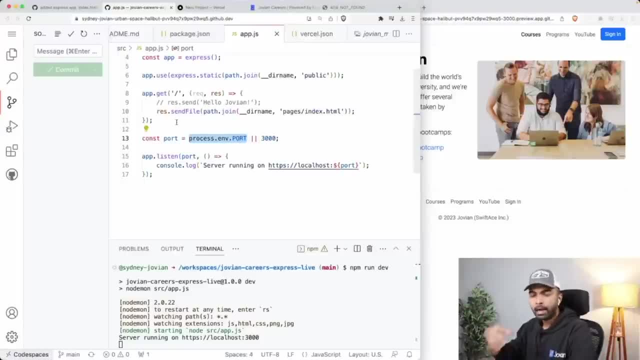 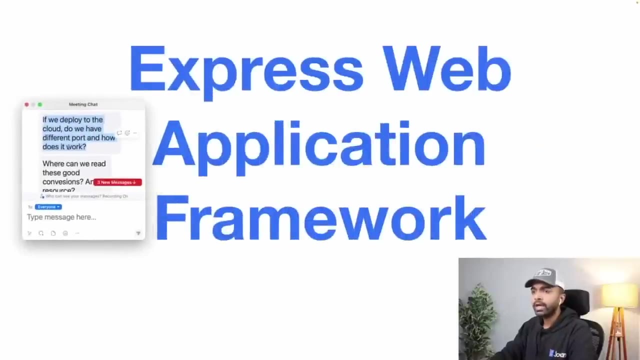 supplies a port number and, ideally, your application should have the ability to read that port number from the environment variable that is being provided by the cloud infrastructure platform, so that it can run on that port. Okay, Okay, Where can we read these good conventions? 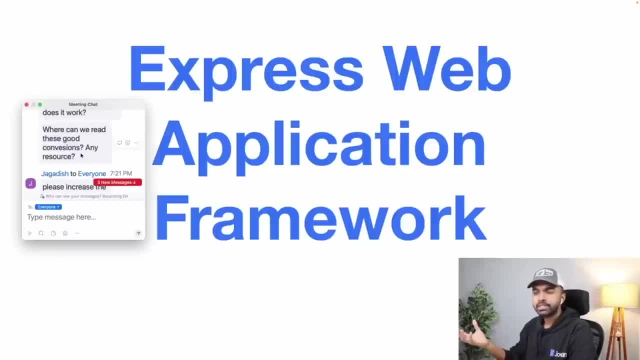 Any resource. Well, these are all just things that you will almost always end up doing. So what we're doing right now is just the only way to do it. You just have to go through the process of building an application and you kind of learn all these conventions along. 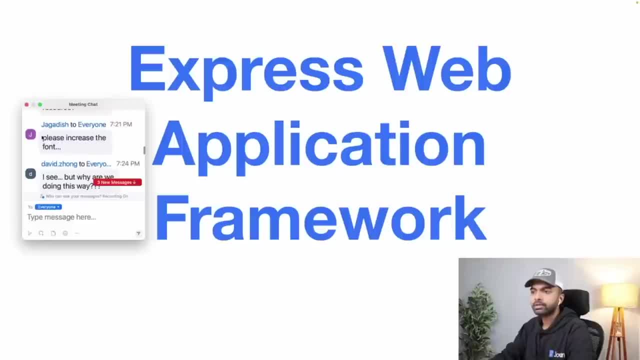 the way. It's hard to go wrong. You can just search these online. How do I do this or that? Okay, Why do we do it this way? Why do we have a request? Why do we have a request, a client and a server? So the client. let's say you have an application like Jovian, which has 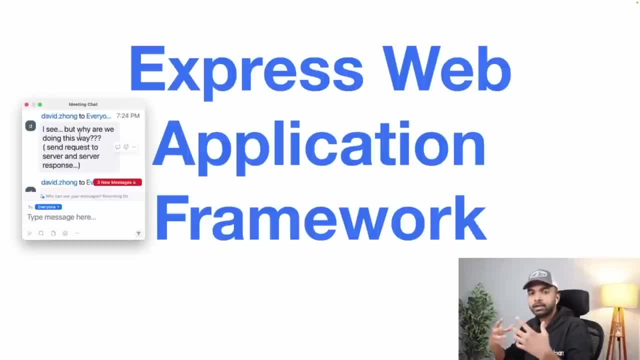 the data of 300,000 users. Now, when we have the data of 300,000 users and you open joviancom on your computer, I don't want you to be able to access the data or access the private data of all 300,000 users. That is why, in your browser, I simply give your browser the ability to contact my 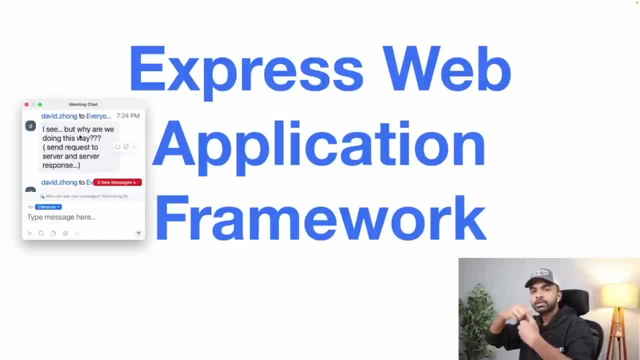 server And then, when your browser sends a request to my server, I have a way to validate: okay, this came from this particular user And then I can ensure on my server that I can contact the database and only return the data that is made. that makes sense for you, Okay, But if I simply 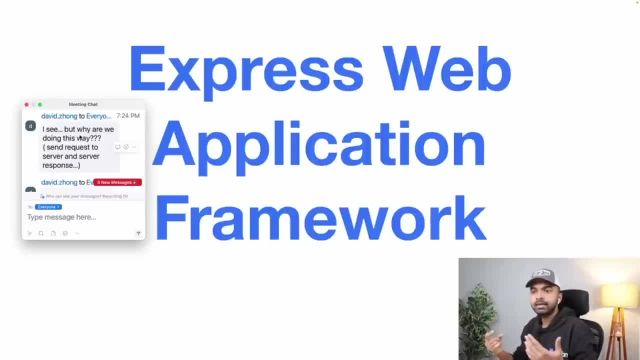 opened up my entire database, then anybody would be able to access anything, And that's why we put a server in between to do this. Okay, what is their name? Well, as I mentioned, underscore- underscore their name is going to say when you use it within a particular JavaScript or Nodejs file. 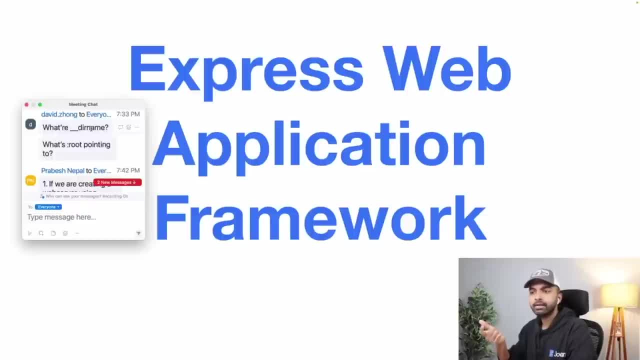 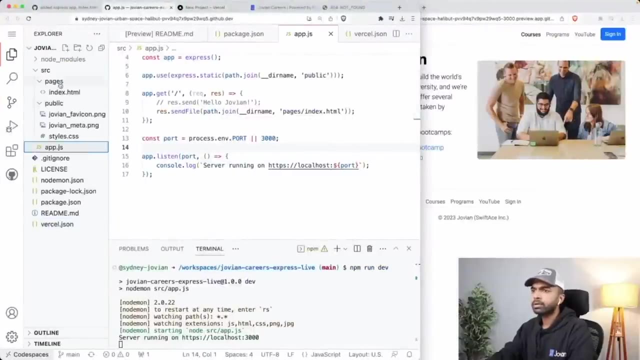 it is simply going to get the directory which contains that file, And we have just used it to get the full path for the pages index, dot HTML, and for the public directory. What is colon root pointing to? Yeah, So in our styles, dot CSS. this is something we covered the last time in our 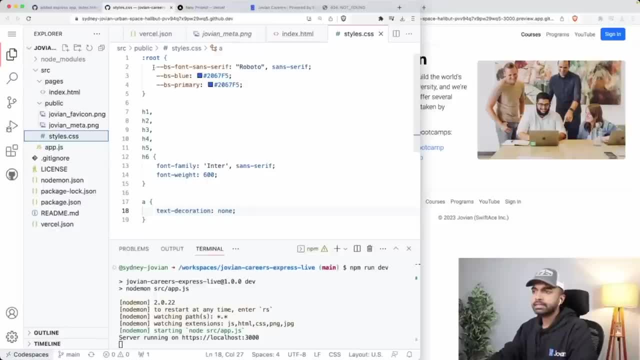 styles dot CSS file. colon root simply is a way to define some global CSS variables. All right and it's good. It's global not just within this file, but across all files. So because we want to override some CSS variables that have been defined in bootstrap. that is why colon root is going to. 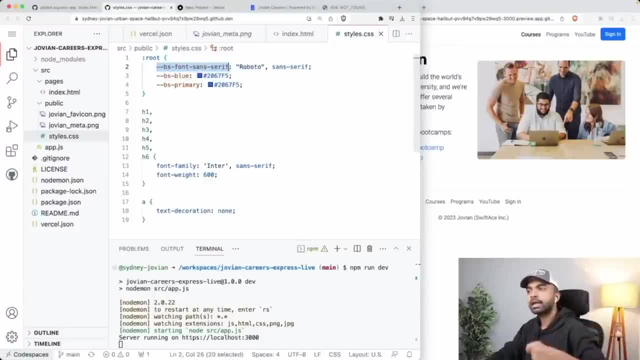 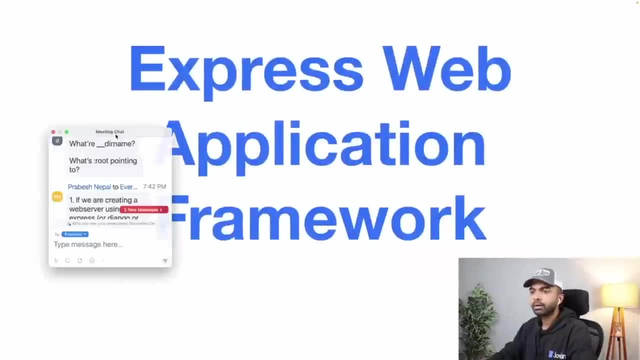 take whatever global CSS variable is there and it's going to rewrite the variable with this name, with this value. Okay, so this is how you override the CSS variable. If we are creating a web server using Express, then what are Apache web server or Nginx or Tomcat? Okay, I will not get into. 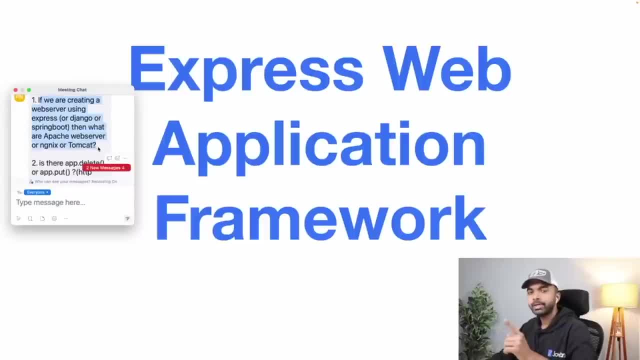 those right now. I will encourage you to ask chat, GPT or job or this question, Or is there an app dot delete, app dot put Yes, So we'll talk about HTTP methods. So you have all of these. app dot get is just the simplest way, where you're simply getting. it's just one of the HTTP methods that. 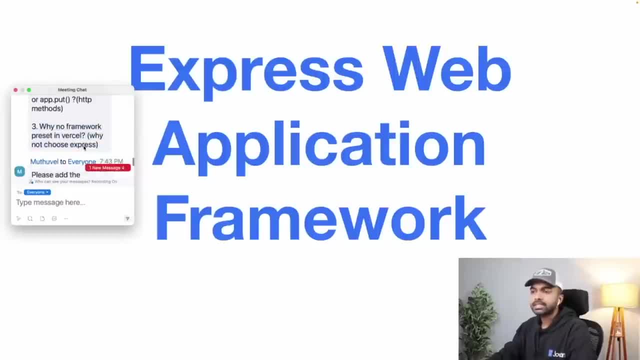 is used. Why is there no express framework preset, and was it for some reason? they don't have it? I'm I guess they should. they should probably have added it at some point, but they decided not to. Okay, please add the questions in the chat as well, when recordings are posted. Okay, 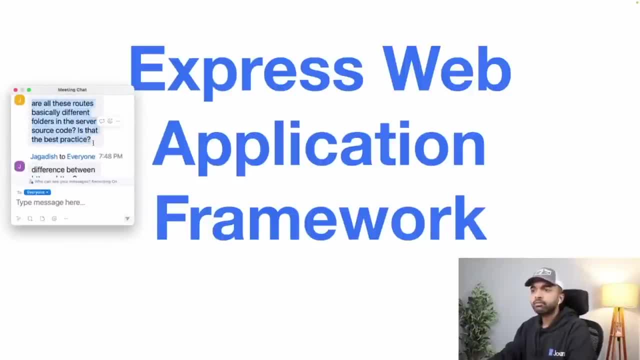 we'll try to do that. Are all these routes basically different Folders in the server, in the source code? Okay, not exactly. So conceptually, yes, as a browser or as a user, I can think of folders. I can think of them as folders on the server. 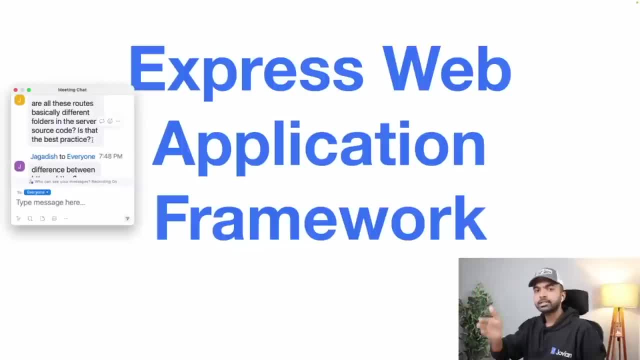 However, if, let's say, we have joviancom slash Akashiness, joviancom slash Siddhant, joviancom slash somebody else, if we create ended up creating folders on our server for every single person, then we would end up with a lot of folders and we would run out of server. 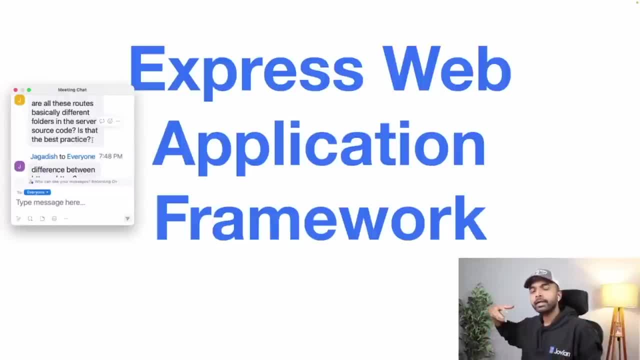 space. What we do instead is we put all the data in a database which is optimized for storing large amounts of data, And then our routes are configured in such a way that, given whatever route we get, they can figure out how to fetch the right. 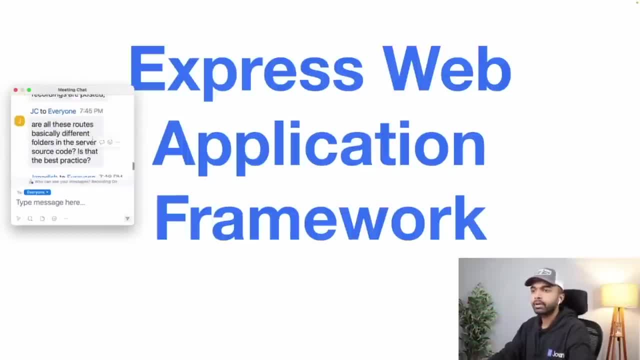 data from the server And we're going to take a look at that shortly. Okay, next question: difference between HTTP and HTTPS. So HTTP traffic is not encrypted, which means if somebody is, can track the packets going going through your network. So basically, 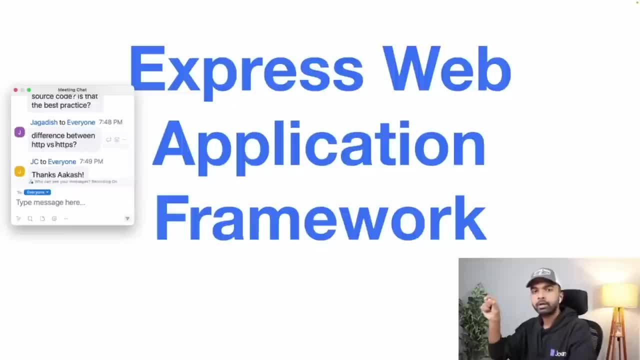 somebody who can kind of listen into your Wi Fi router, or maybe even your Wi Fi router company or internet service provider. everybody can see exactly what you're sending, the full contents that, the email that you're sending, or the password that you're sending, whatever it is. 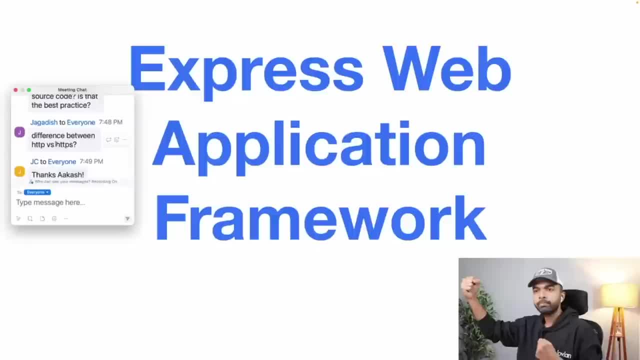 but https means that the client and the server, they have initially done some kind of an encryption handshake and the client encrypts the data, sends it to the server and when the server sends back the response, it encrypts through the data, sends it to the client, in the client being the browser. 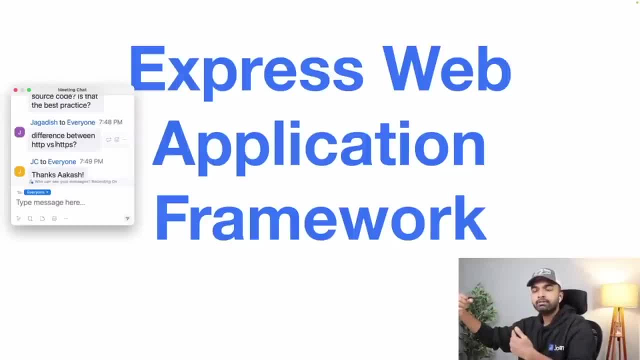 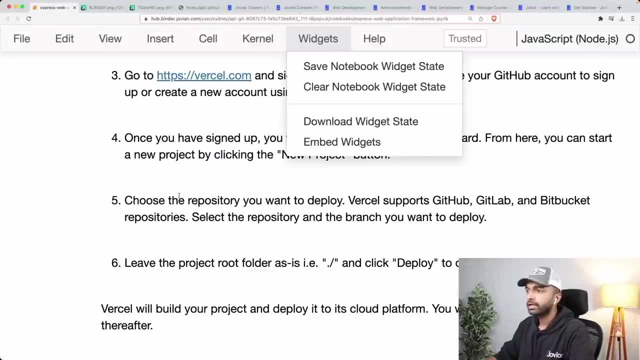 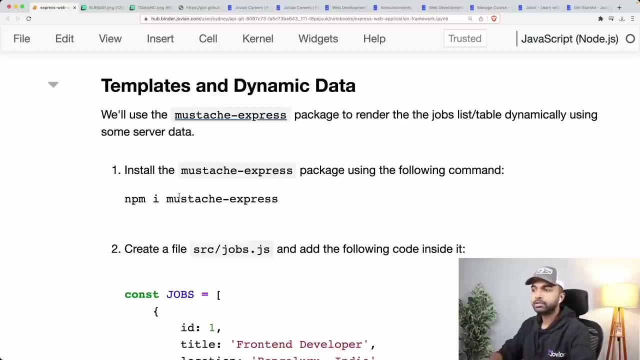 in between. your internet service provider or somebody just listening into your wi-fi will not be able to see what's going on. and now most websites just work on https. so, moving right ahead, let us now send some dynamic data and add it into the indexhtml page. 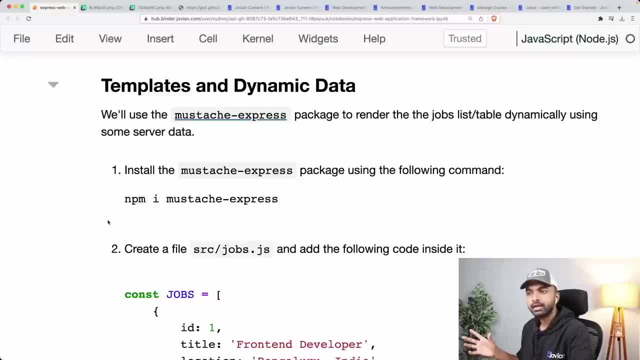 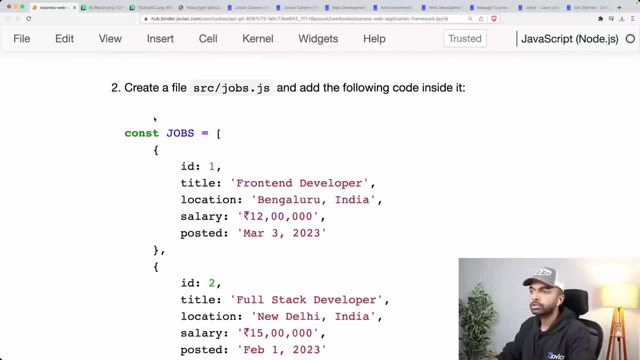 now, of course, we are not going to talk about databases just yet, but we are going to simulate databases in a certain way, essentially. so here's what we're going to do: we're going to create a file called jobsjs. so i'm going to create a file here called jobsjs. 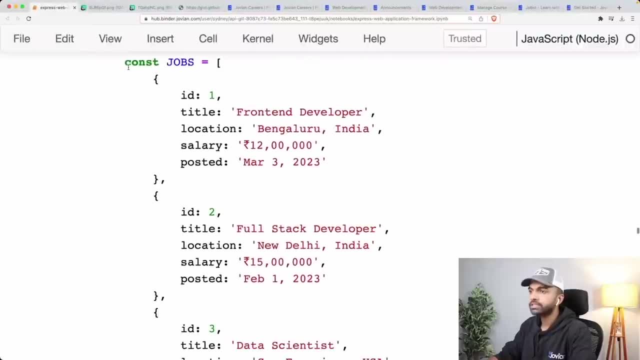 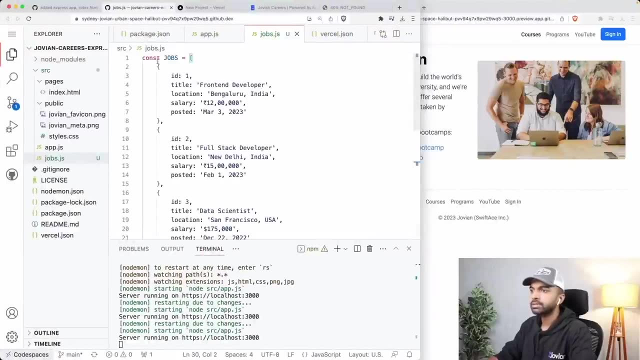 okay, and in this jobsjs file i'm going to put in some data. let me take in all this data over here. and this is simply a list of jobs. so cons, jobs equals. this is our first job object which has an id, one title: front-end developer location, bengaluru, salary 12 lakhs. posted on march 3rd 2023. 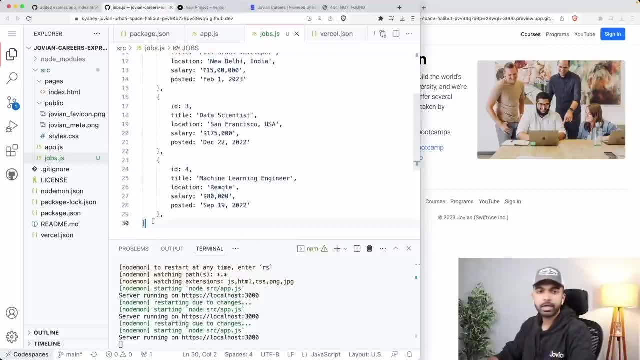 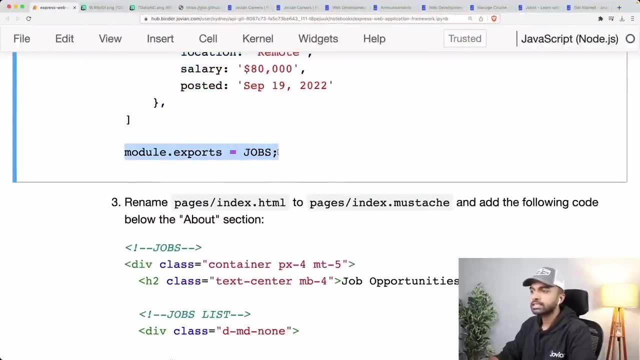 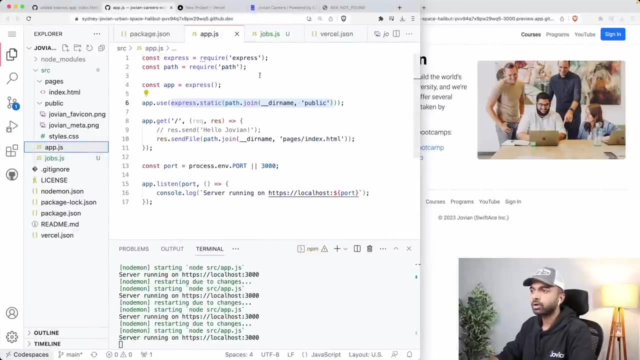 similarly, there's a second job, third job. so we've taken a json array, an array of json objects, and put that into this variable called jobjs, and, uh, we are going to just export this as the default export from this module. okay, so jobsjs is this file into which we have put in a bunch of jobs. now, um, we can actually import these jobs. 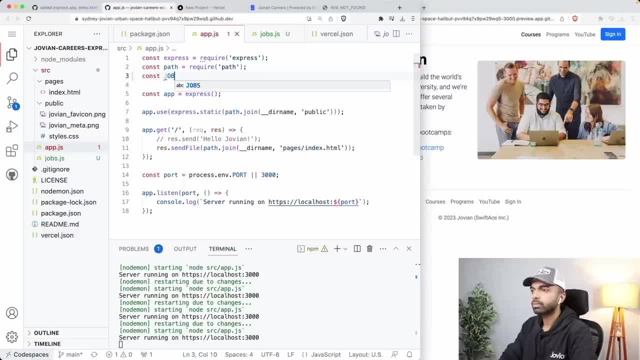 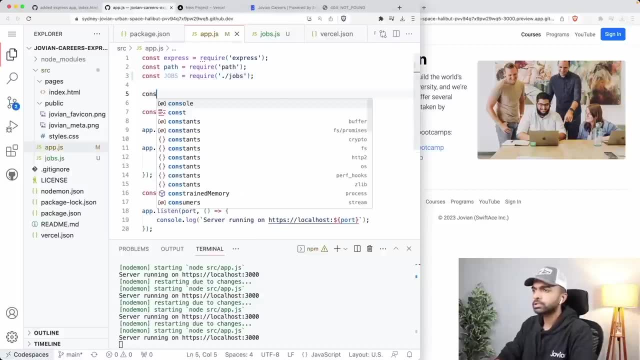 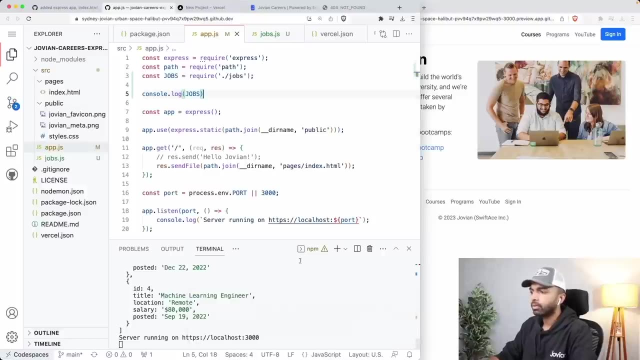 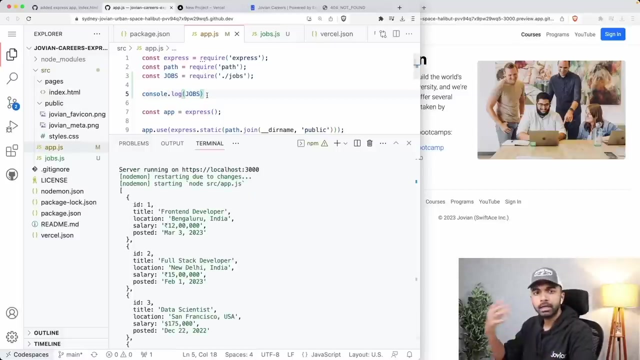 here, so we can say const jobs equals require dot slash jobs. okay, and i can also just consolelog jobs, and you can see that when we import this from require dot slash jobs, we get all of this data here and we can now use it in our server and we can even send it to the browser however we want. 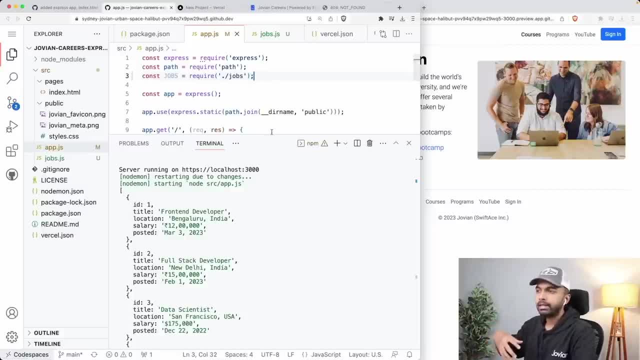 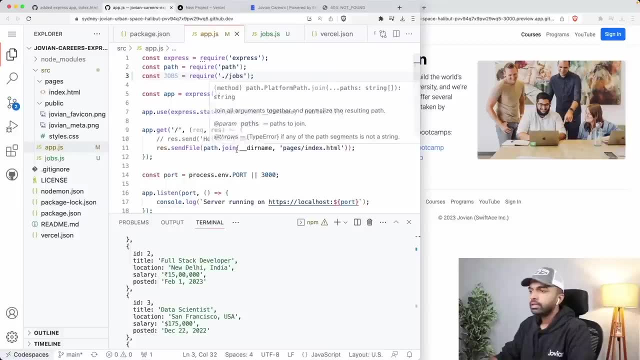 okay now, of course, right now, we are getting this from a file, but in a real world scenario, you would be getting this from a database, which is something that we'll look at in a future course. okay, the next thing is to actually put these jobs into the indexhtml file, so we're going to import these jobs. 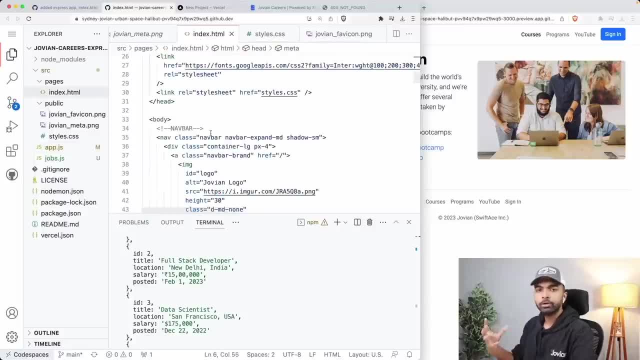 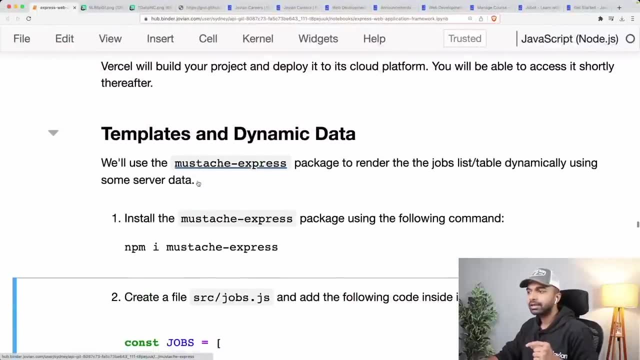 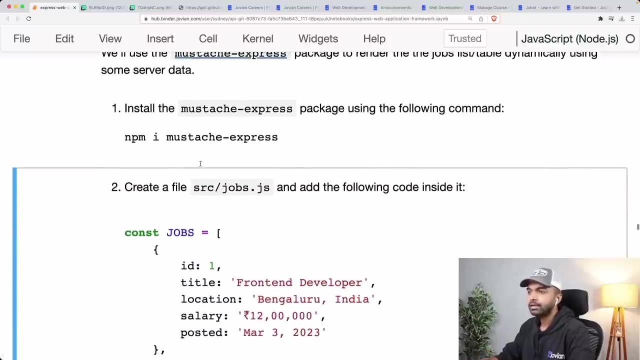 into the indexhtml file. so now what we're going to do is turn this indexhtml file into a template, and we're going to turn it into a template using a template rendering system called mustache- and i'll talk about what mustache is in just a second. but here's what we need to do. 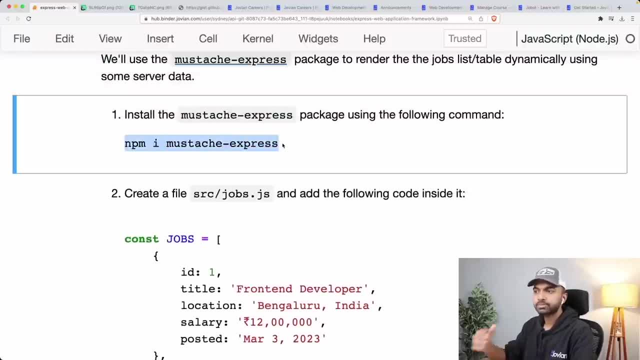 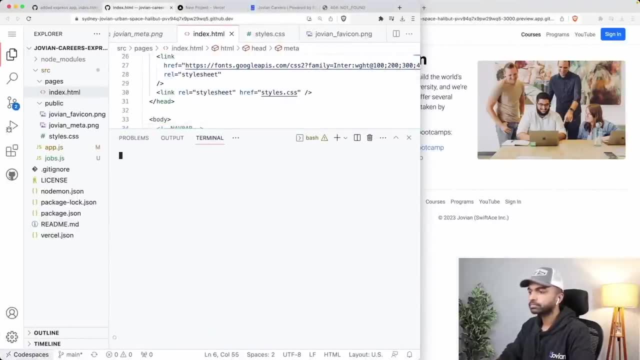 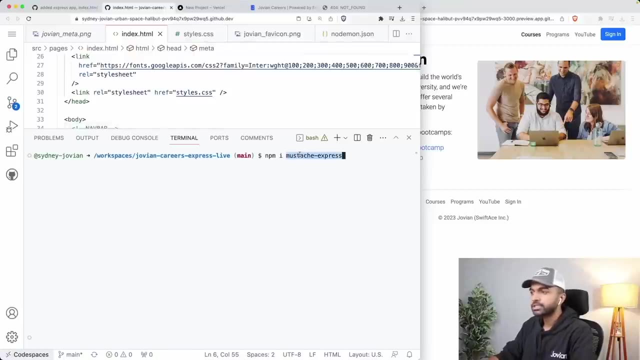 the first thing we need to do is install this mustache express package. so i'm just going to go in into the terminal and i'm just going to stop this server for now. i'm just going to say: npm, install mustache express. so mustache is the templating, the template engine that we are going to use, and mustache express is. 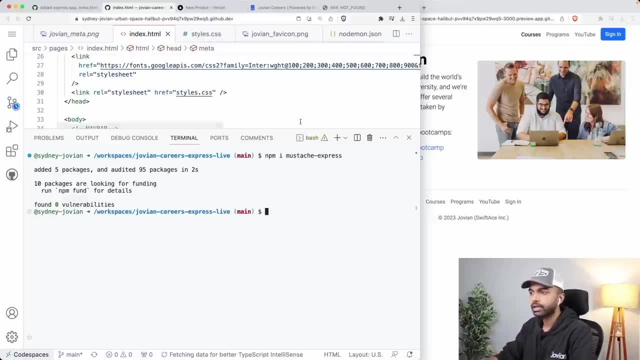 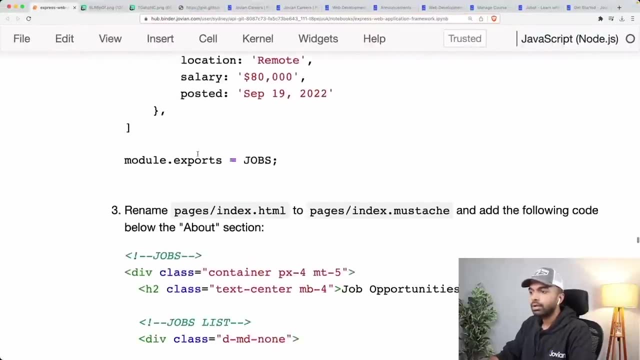 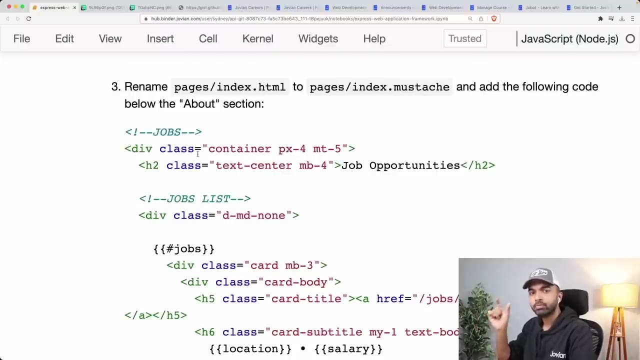 the connector that that allows you to connect mustache to x, allow express to mustache. okay, so that was step one. the next thing we need to do is to convert our indexhtml file, which is an html file, into an indexmustache file. indexmustache file or a mustache template. 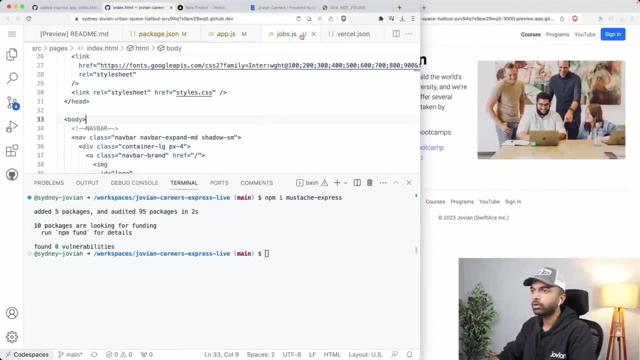 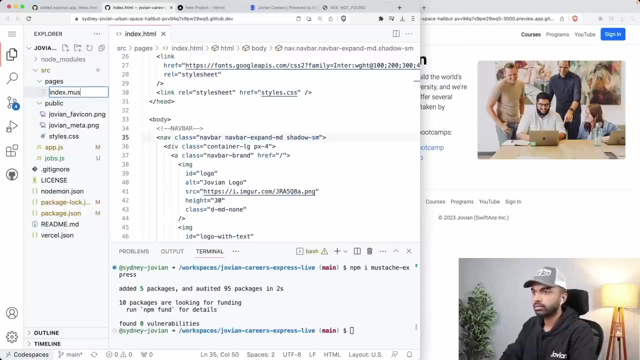 Okay, And here's what we're going to do. So I'm just going to go into my indexhtml file And I'm simply going to rename this file. So I'm just going to rename this file to indexmustache, Okay. 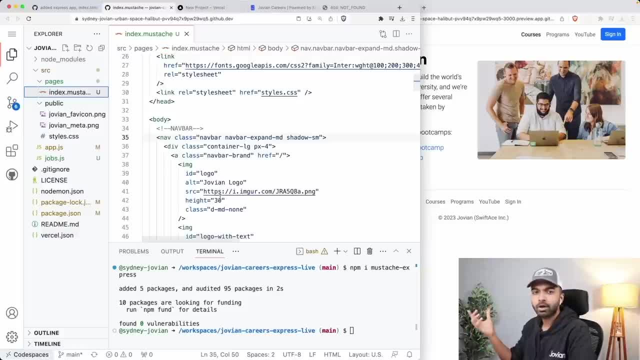 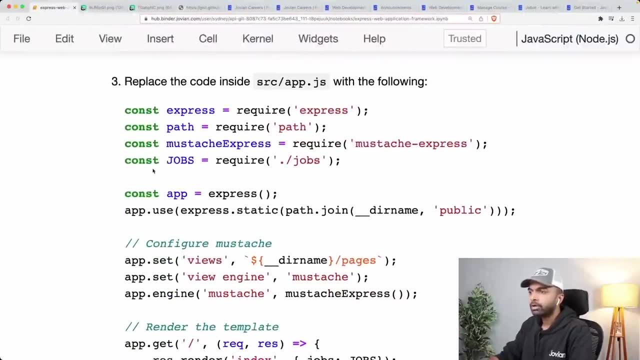 All right, So far, so good. We've not really changed anything. We just installed a package, renamed the file. What difference does that make now? Um, we'll add some of this later. Now I'm going to come into my app file, my app server, and I'm going. 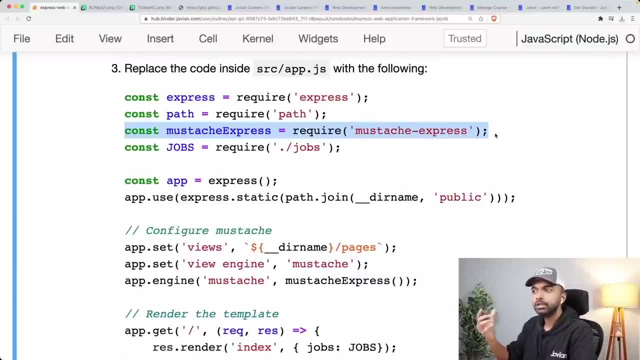 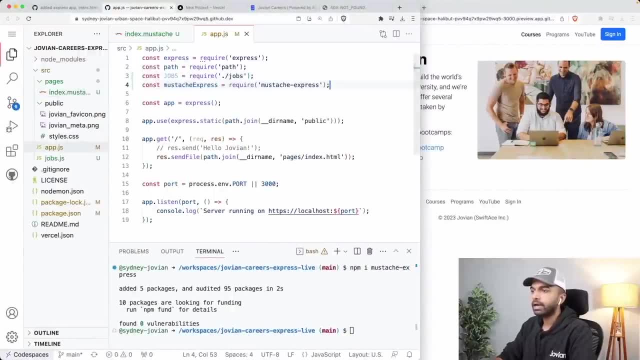 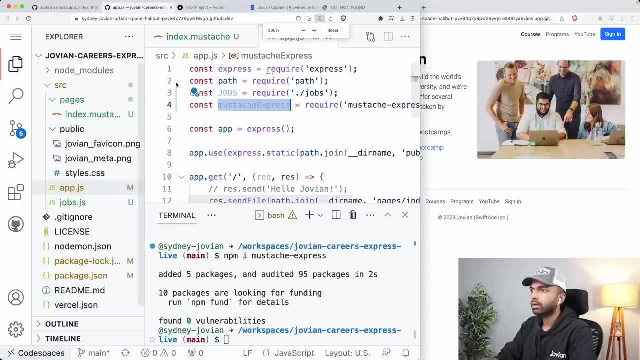 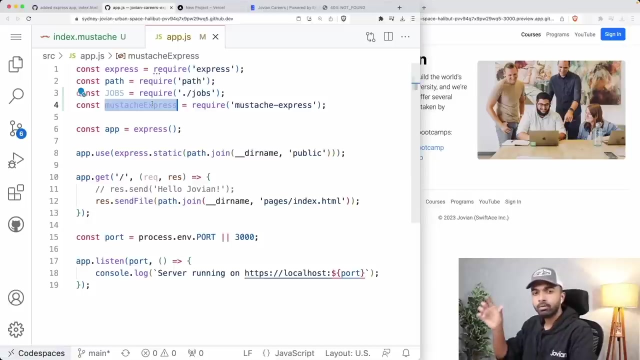 to incorporate the mustache template rendering engine into my express server. So first thing I'm going to do is go into appjs and just require mustache express and get this mustache express object. Okay, So now I have this mustache express object over here and in this object- uh, this object now. 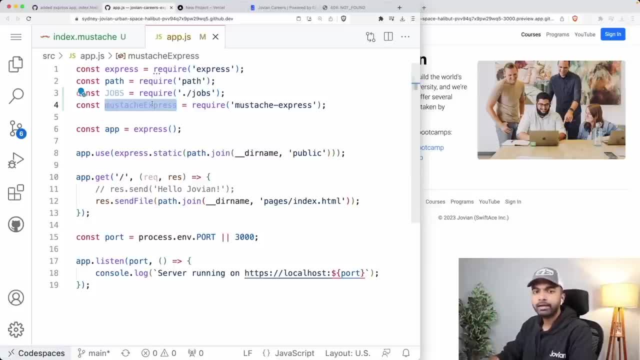 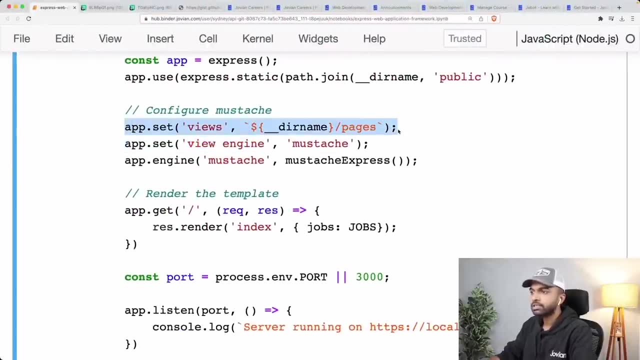 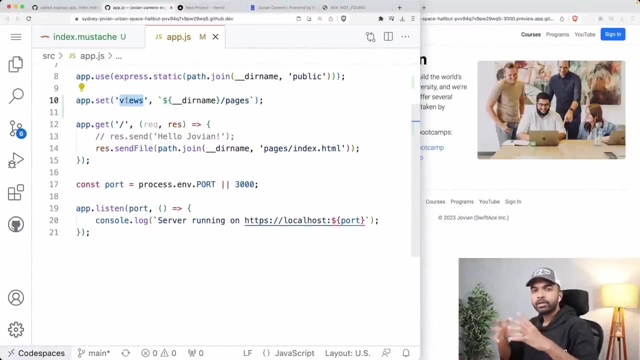 contains the mustache template rendering engine. Now I need to add it into my app express app, and the way we add it is like this. So first we have to set a bunch of views within our application. So what we say is that the views or the templates or wherever whatever, contains the markup or the 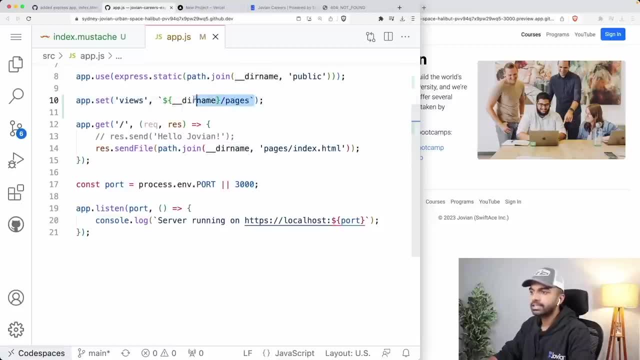 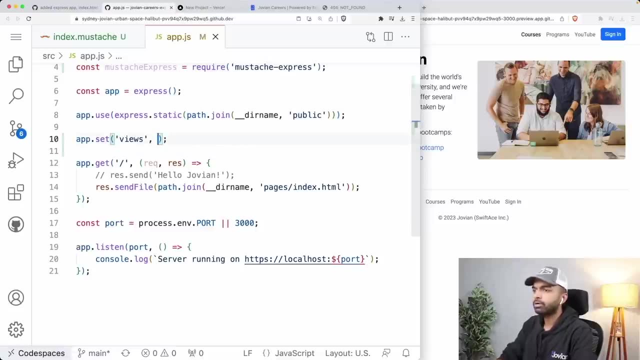 HTML Is all present inside this folder called pages. Okay, So what we're saying is: um, let's actually just make that nicer here. So what we're saying is: app dot. set views to path dot. join underscore. underscore their name pages. 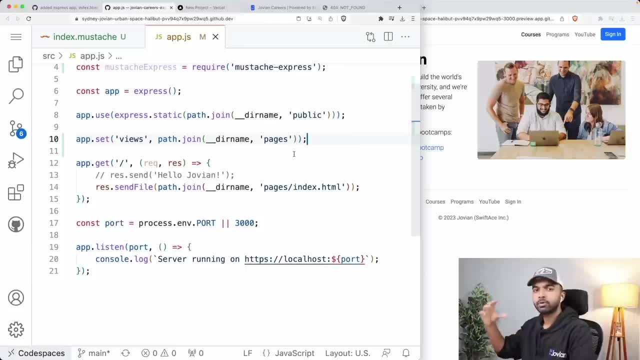 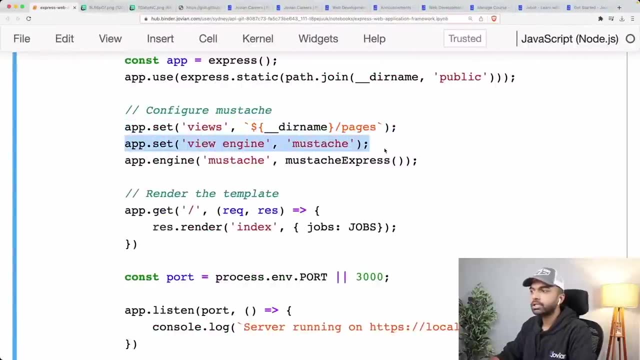 All right. So we are saying that inside the pages folder I have a bunch of views or I have a bunch of templates that I can use. Uh, that's the first thing. Second thing we need to say is that we need to set the view engine. 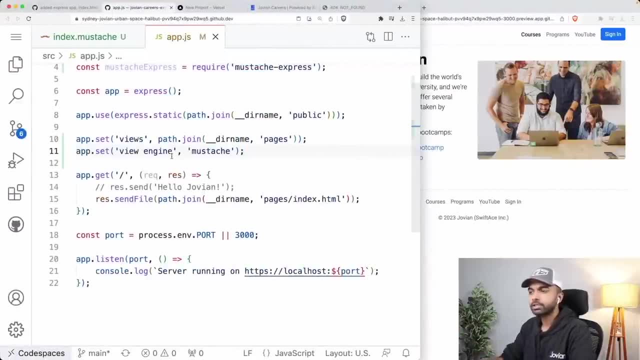 Okay, Whenever you hear view, think of it as template. These are all just words for the same thing. Um, so now we say: app dot, set view engine to mustache. Okay, So we've set a directory that contains our templates or our views. 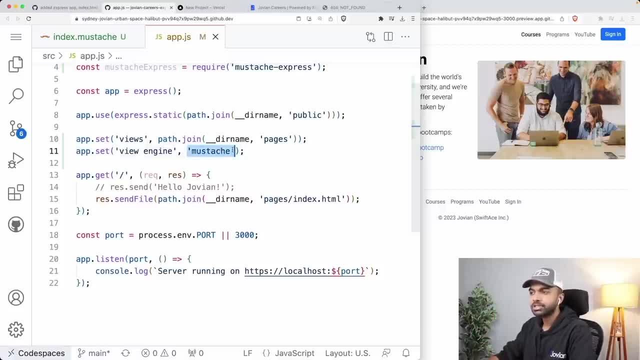 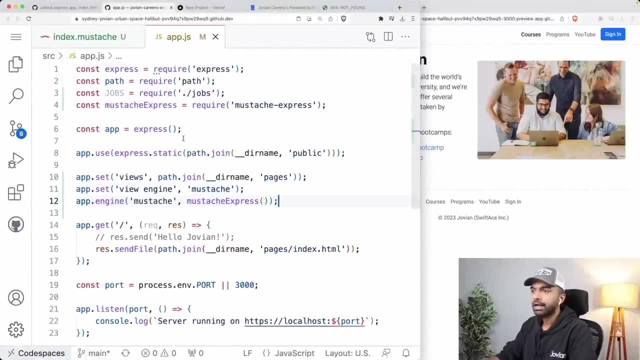 Then we set a view engine and that engine has the name mustache And finally, for that engine, we need to provide the handler function. Okay, And the handler function is simply coming from mustache express, All right, So, uh, three things we need to say. 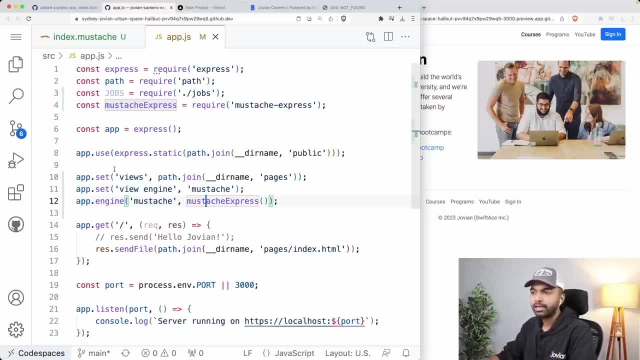 Anytime you're adding some form of templates to render some form of dynamic data, and all of this will become clear When you actually see this in action. you need to set the views. So the views we are simply setting to the pages folder, you need to. 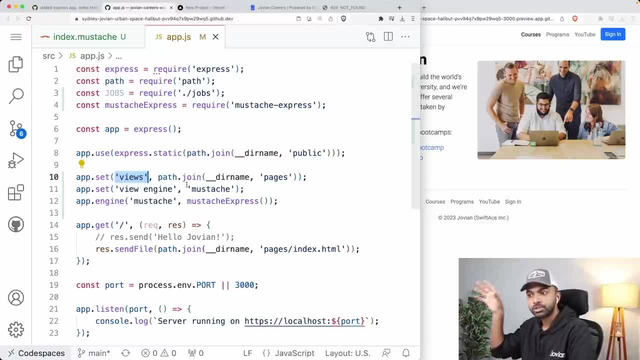 set the view engine and the view engine. We are simply setting uh to mustache and the actual engine that we are using for the engine name mustache is called mustache express. All right, So this is just something that you'll have to drop into any express. 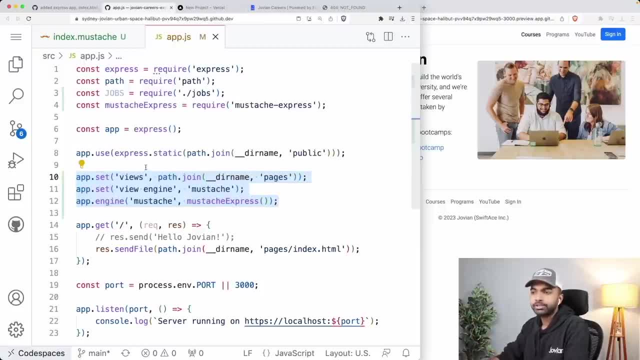 application whenever you're adding some some templating uh engine to- And there are a bunch of other templating engines as well, like bug, EJS, et cetera- Mustache is just the easiest one to work with, a really simple to understand. 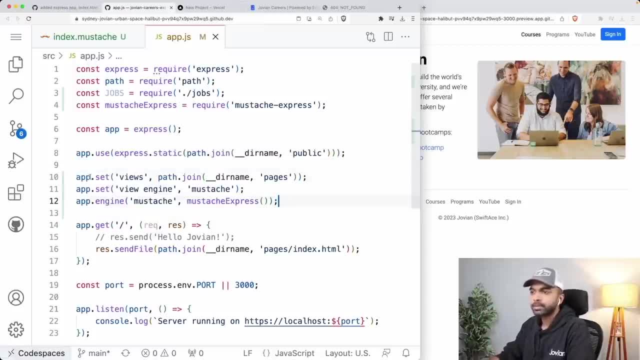 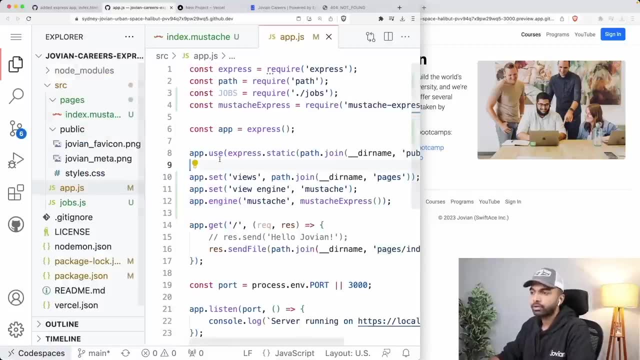 All right. So so far, we have installed mustache express, set it as the view engine and we've said that all our templates, or mustache files, are inside the pages folder. Okay, Now the next thing we can do is we can go in and render that template. 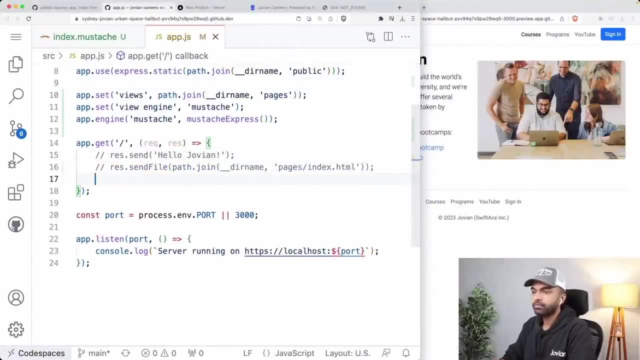 So here's what we can do: instead of saying rest dot send file, which is what we were saying Earlier, we can say rest dot render And, in while we are rendering, we need to give it the name of the view that we want to render. 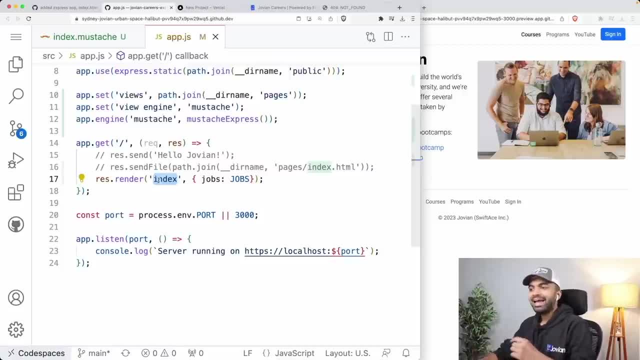 So we are saying that we want to render the view index and we want to send this data into that view, to populate the uh, to populate that view. Okay, Again, these words will soon make sense, but basically now you can understand that. 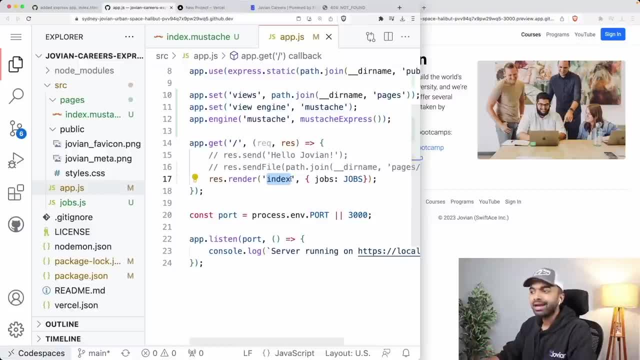 Okay, Index simply refers to the index or mustache file, and that index or mustache file is going to be located in the Folder That has been configured for reviews and the folder folder is called pages. All right, So we have this: pages folder index or mustache. 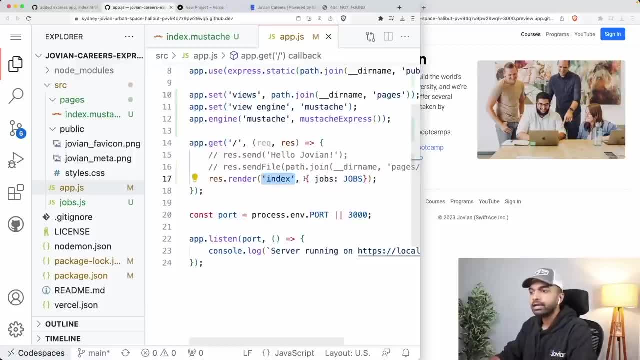 So so this is simply going to pick up the index or mustache file and it's going to give this additional data, which is a dictionary containing the key jobs, which points to the list of jobs that we have, And that additional data can now be used within our index dot mustache template. 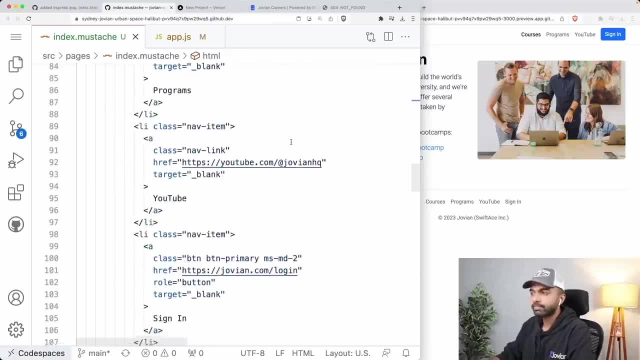 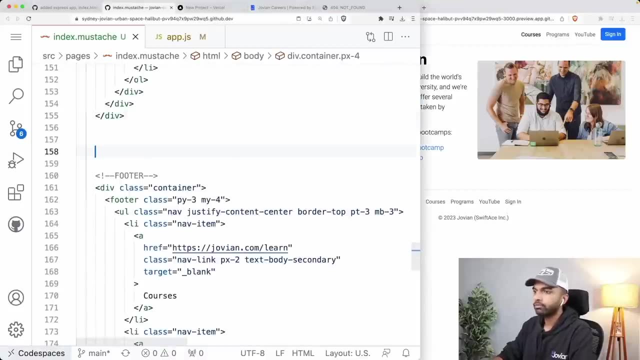 Okay, So let's come back and actually use this. Now we have in this page, we have this about section And then We have this footer. just below the about about section and above the footer, I'm going to add a new section called jobs. 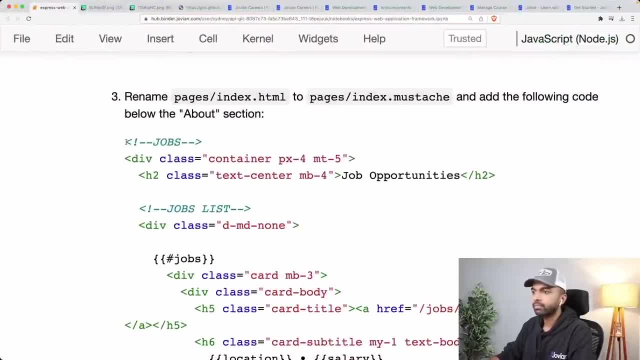 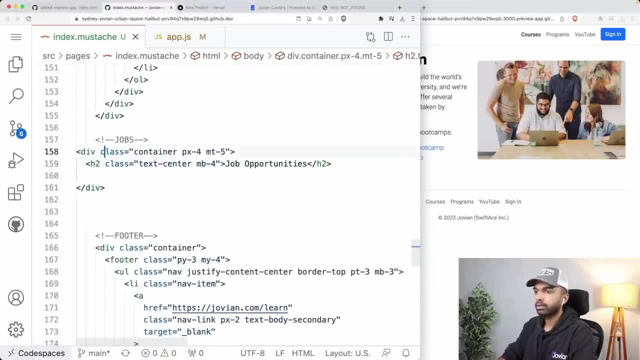 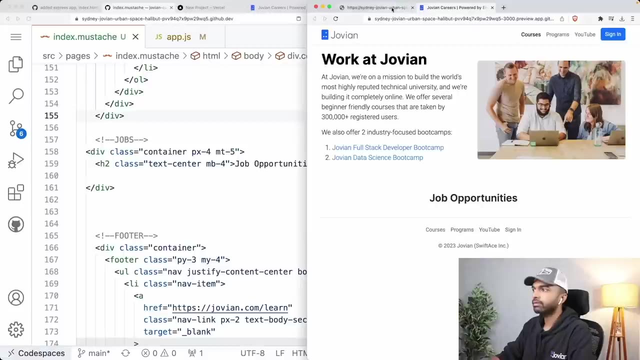 So here's what I'm going to do. I am going to first add this div, or jobs, job opportunities. Okay, So so far, there's nothing new we've done. We've simply added this job opportunities div, and there we have it. 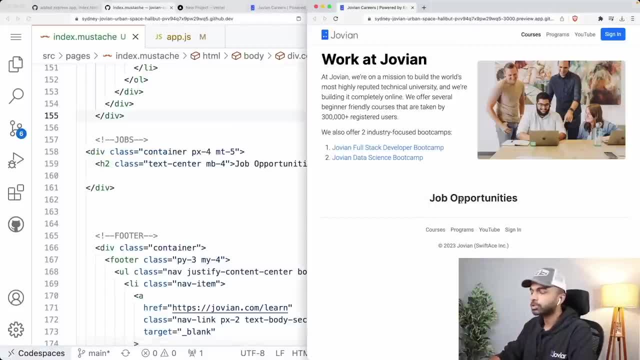 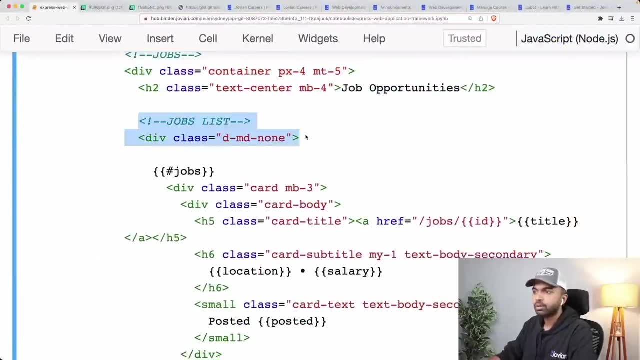 Okay, So now we've simply added a simple div which says job opportunities. Nothing fancy going on here, but then we want to now add the job list, So let's add this jobs list. So this is going to show up only on mobile. 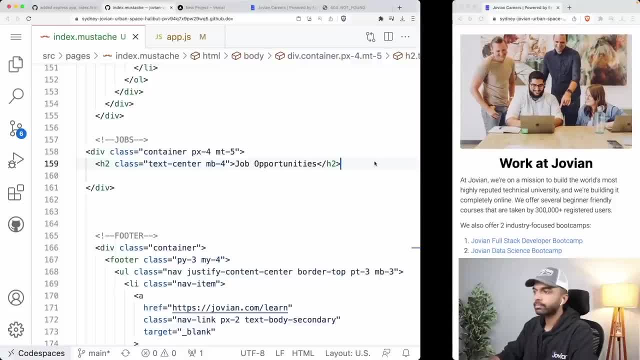 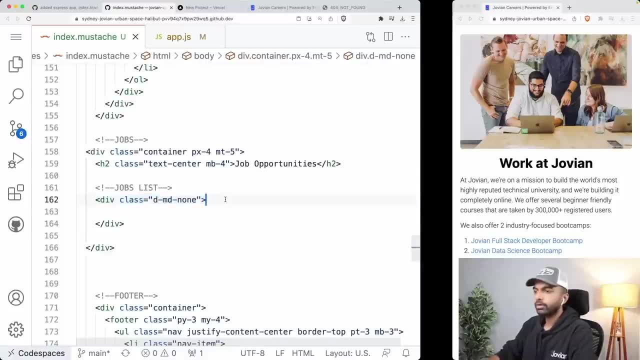 So I'm just going to reduce the width over here as well so that it shows up properly. So this is going to be a jobs list and let's add the slash div over here. Okay, Now, inside this jobs list, I'm going to do something very interesting. 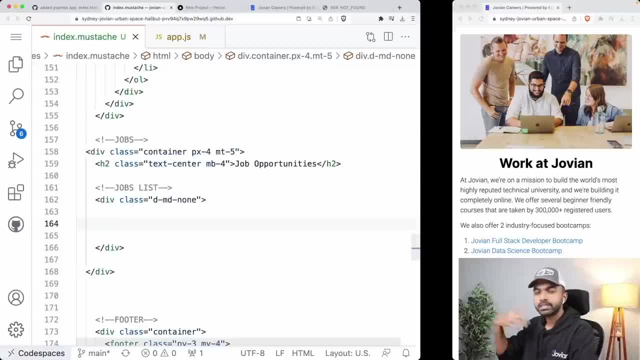 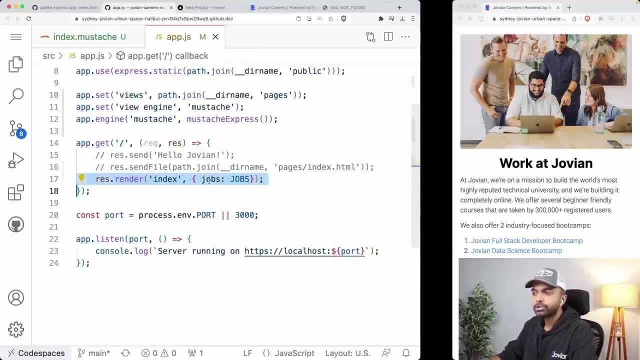 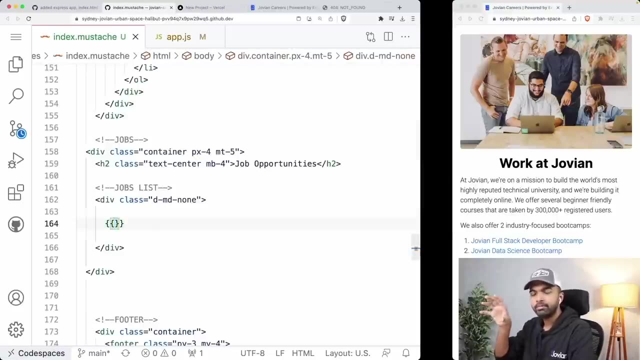 I'm not going to type out all the jobs one by one, but instead remember that my template, It is being rendered with this data, So I have access to a variable called jobs which points to a list of jobs. Okay, So I, so I can take that list of? uh, I can take that variable which is a list, and I can loop over that variable like this: 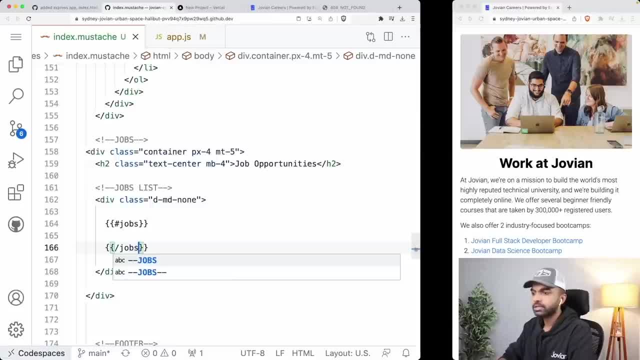 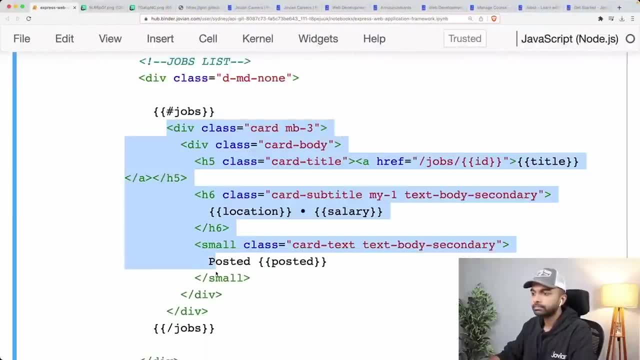 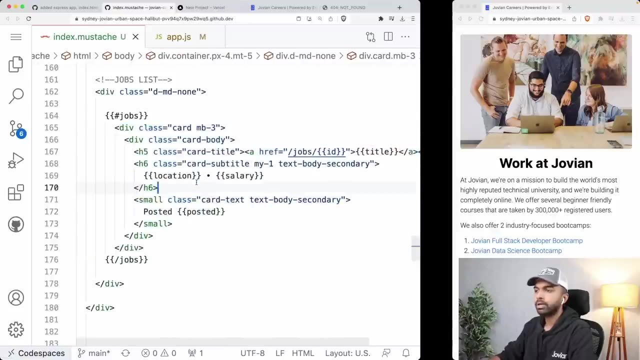 I can say: hash jobs, slash jobs. So what this is doing is, this is basically creating a for loop and inside this for loop I can put in this content Like that, So I can say, okay, so let's see what is happening here. 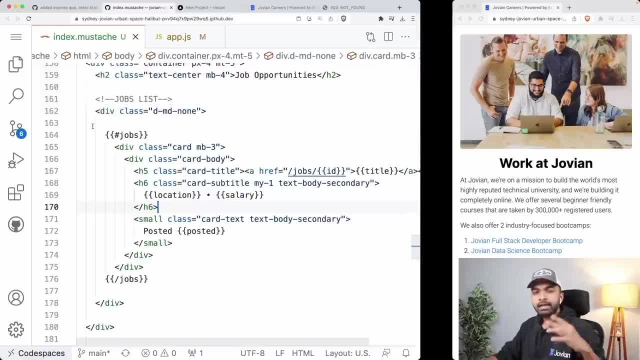 So let's see what is happening here. We have it. We had an index or HTML file. We just renamed it to index on mustache. inside it We added this new div called jobs list. inside this jobs list, If we use this special syntax called bracket bracket, and that's why these are called the mustaches or the curly braces- 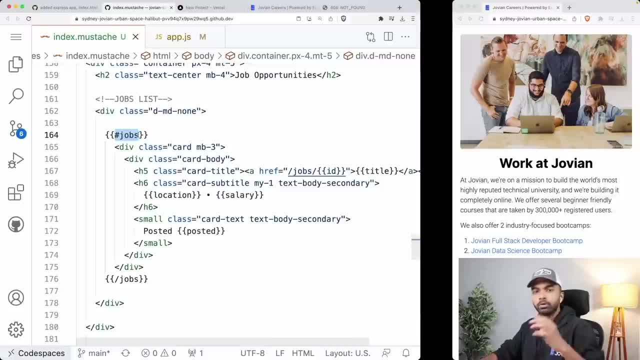 That's why the library is called mustache. And then we said that, okay, we want to look for this object or this key called jobs and whatever is there in that key. If That is a list, we want to loop over that list. 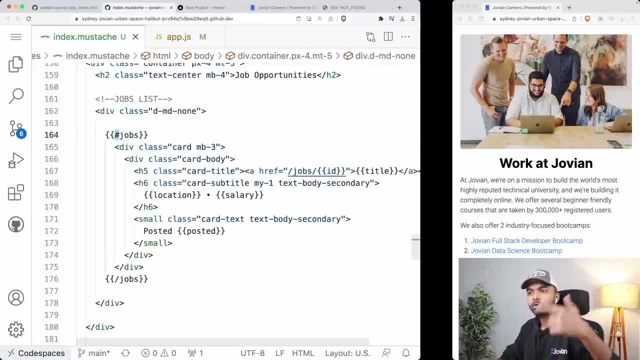 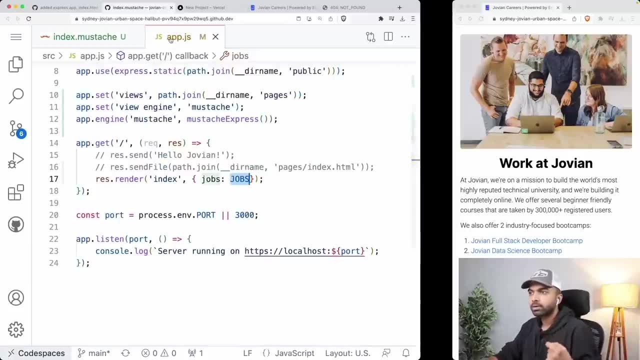 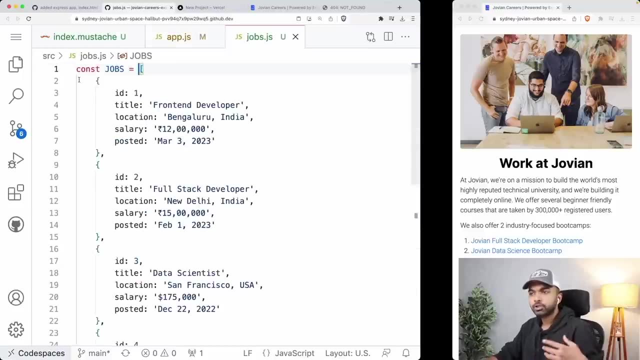 And that is where we use this hash character. This hash basically means we want to loop over something, And this slash simply means we are. we are at the end of the loop and then in each loop. So remember our jobsjs file. our jobsjs file contains a list of jobs. 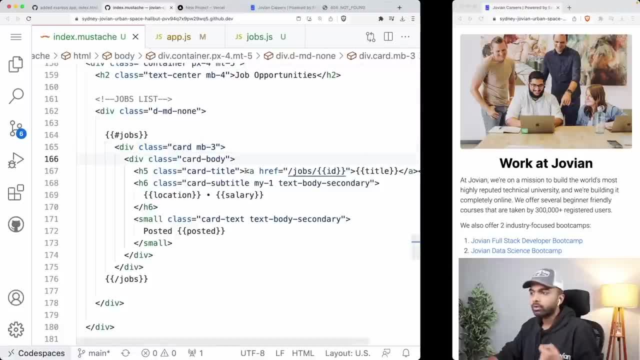 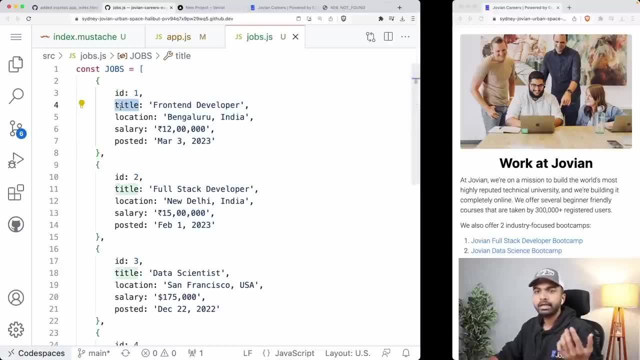 So in each loop we have access to the job, And now what we can do here is we can use a particular key or a particular, a particular key from the object, For example, a key, For example. we have the key title. 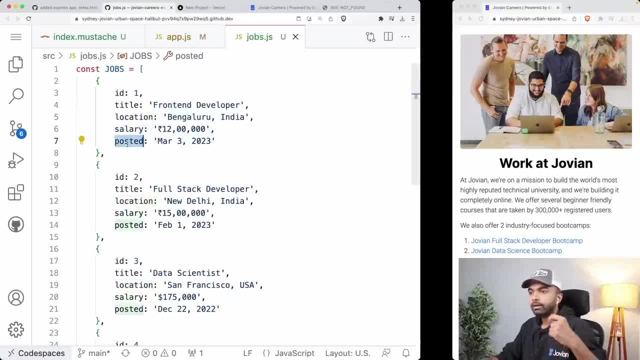 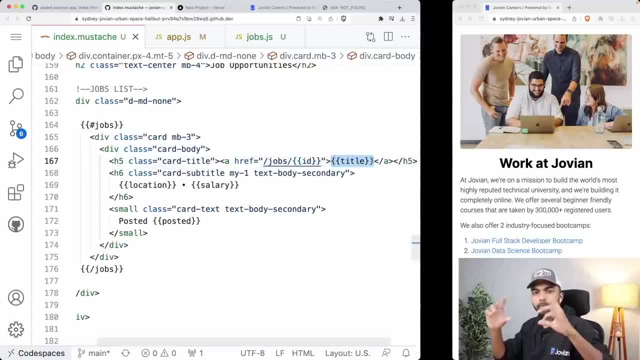 We have the key location, We have the key salary, We have the key, We have the key posted. So all of those can now be accessed within this loop. Okay, So now, bracket bracket, title: bracket bracket is going to get the value for the first element in the first loop. in the second loop, 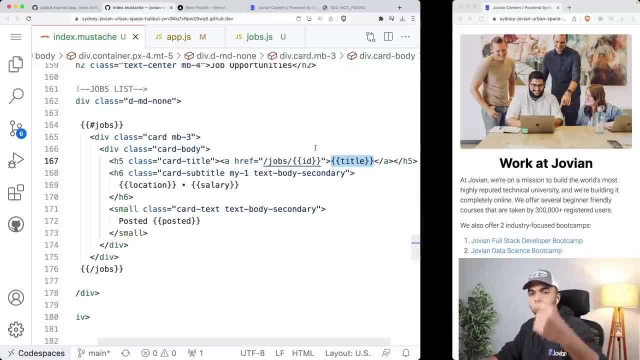 It's going to get the value for this for the title from the second element, then it's going to get the title from the third element, and so on. So, because there are four jobs listed here, Four of these devs will Be rendered div, div, div, div, and in each of these four divs, the data from that corresponding job will be picked up. 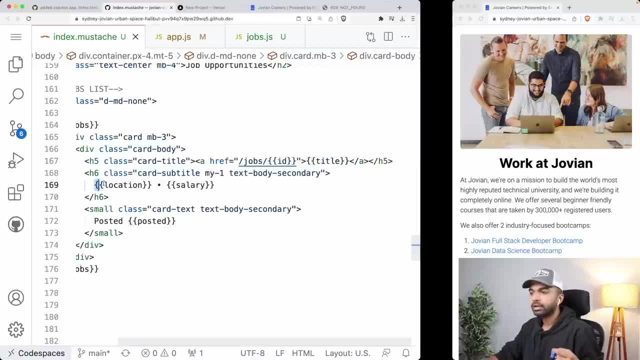 And what data are we picking up? We are picking up the title, We are picking up the location, We are picking up the salary and we are picking up the posted. Okay, So wherever you see bracket, bracket, that is going to get replaced with some actual data. 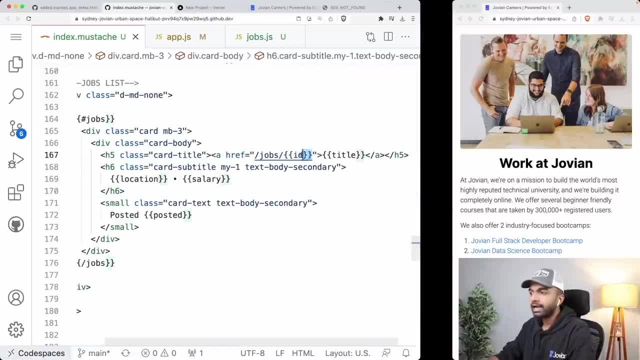 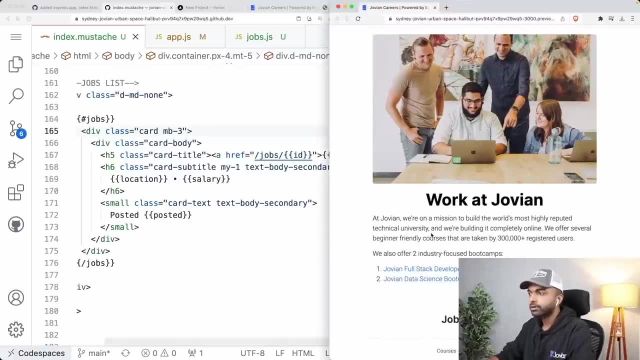 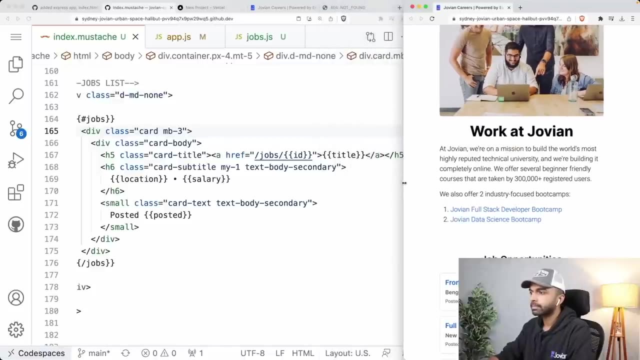 And finally, we are also picking up the job ID and using that, we're creating a link. Okay, Let me save that And again, I encourage you to just run this Yourself and see if you can make sense of this and let us yeah. 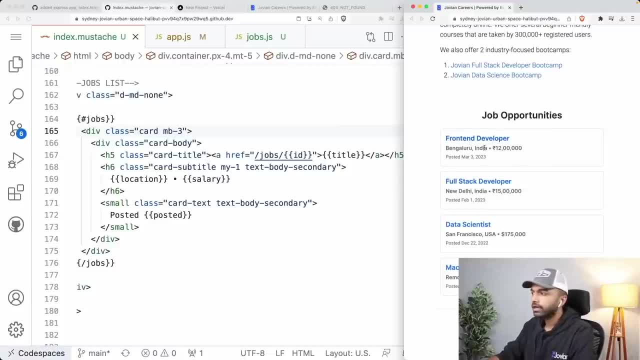 And now you can see here: Now we have job opportunities: front-end developer, full stack developer, data scientist, machine learning engineer, All right. So again, think about what happened. What we did was we installed the mustache express package. 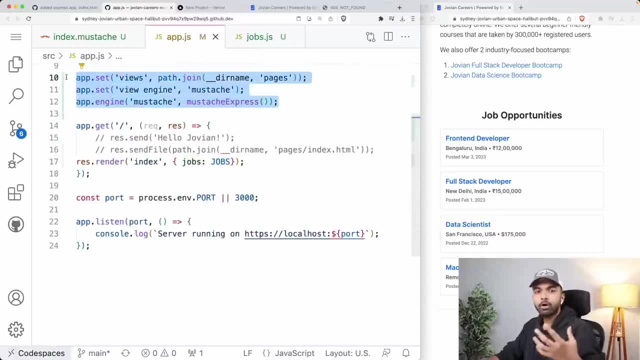 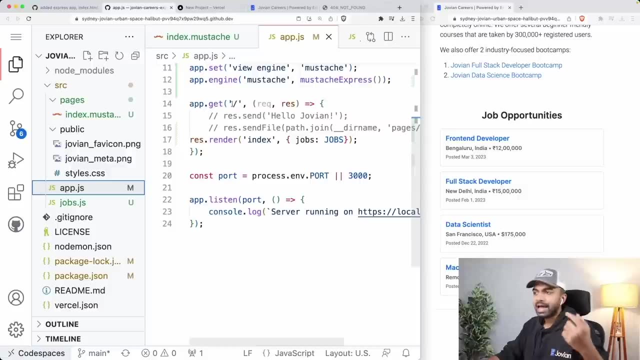 We then imported it, We configured it as the default view engine for express and we configured the default view Direct As the pages folder. then in the slash route we are simply rendering the index mustache file or the index mustache template into that template. 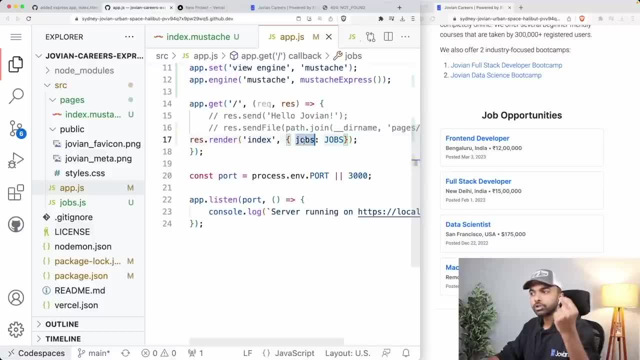 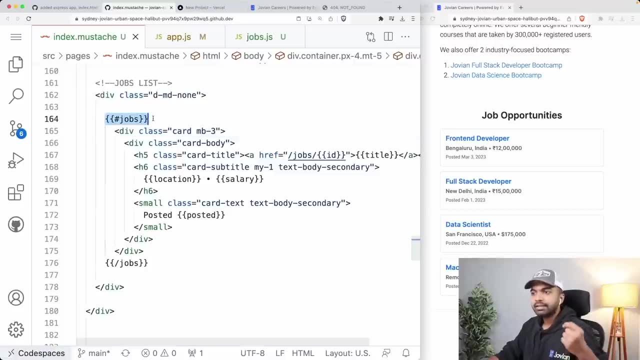 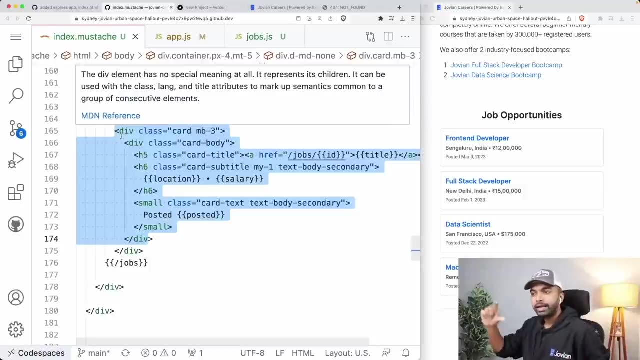 We are passing a dictionary. in that dictionary We have a key called jobs, which is a list of jobs. Now, whenever you have a list, you can use it within that mustache template like this to loop over that list and whatever you put inside the hash and slash that is going to be applied to each element of the list. 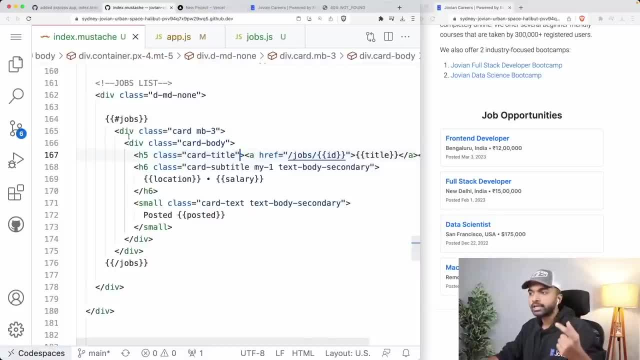 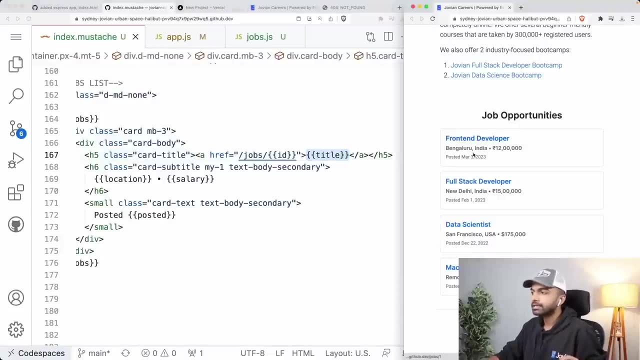 Okay, So each element is going to be one job or one job object. from that one job object, We want to insert into our HTML the title, the location, the salary. So that's why this title gets inserted, The location gets inserted. 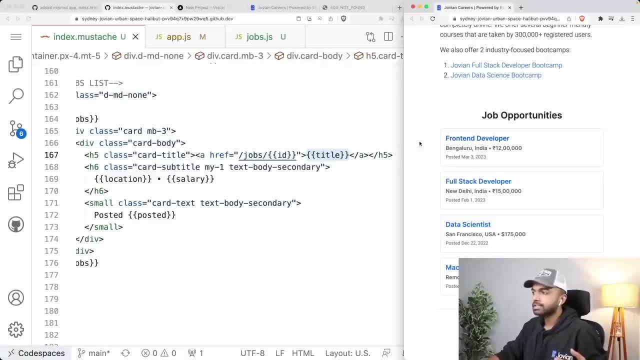 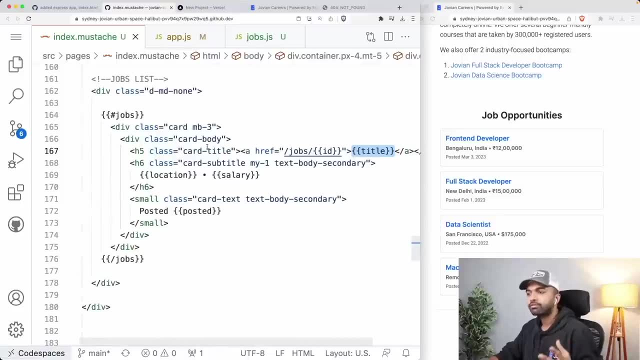 The salary gets inserted, The posted gets inserted and all of this gets looped four times for each of the jobs that we have. Okay, So here this data came from a file, but this data could instead have come from a browser, from a database, or could have come from a third party source like Twitter or something like that. 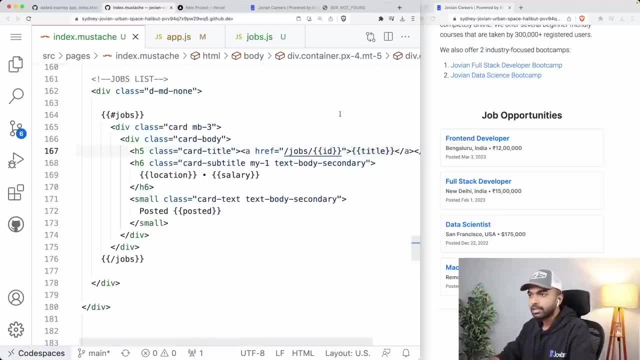 If you are using a Twitter API or something, Okay, So think about this. but this is basically what mustache or any templating engine, is used for: to insert data into an HTML template and fill it out and create a proper HTML page out of it. 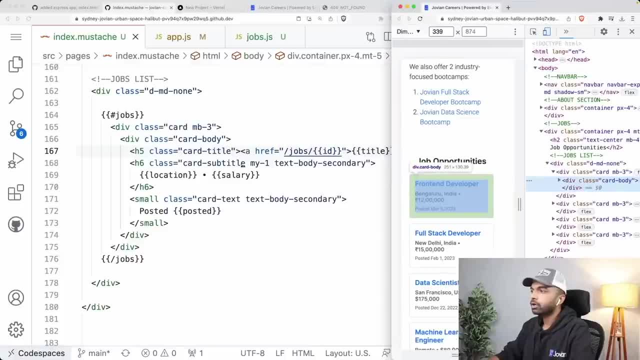 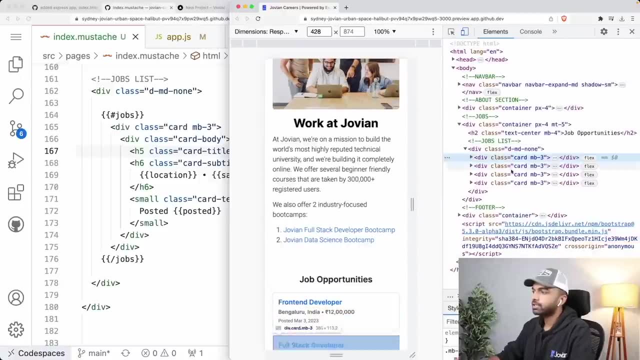 Now, if you just right click here and click inspect, you will not be able to see this template over here. What you will see instead is that we have this jobs list And in this jobs list we have these four jobs, these four cards, and in these four cards we have each of these particular 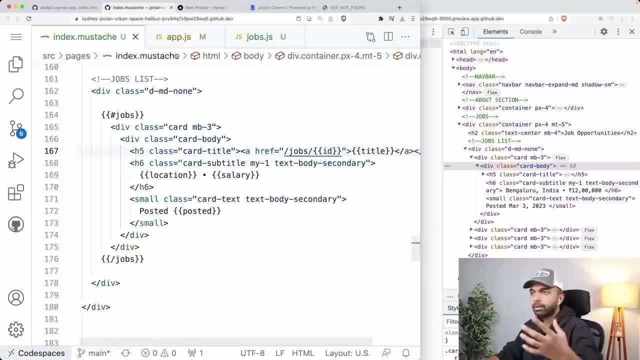 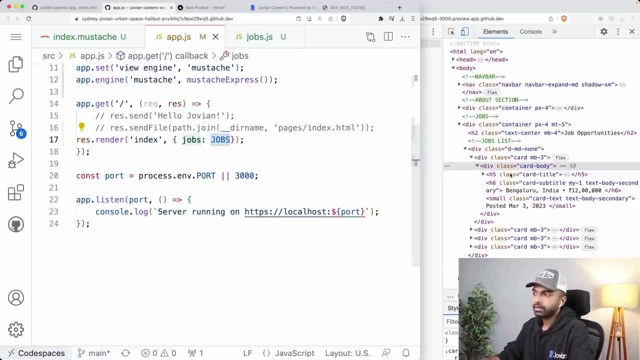 No Data for each of these particular job roles. Okay, So the, so this template, combined with the code that is running over here, is going to generate the HTML and only the HTML, the final HTML sent to the browser, And that is how things work. 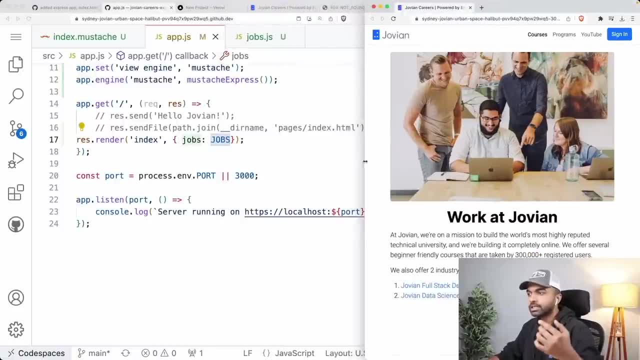 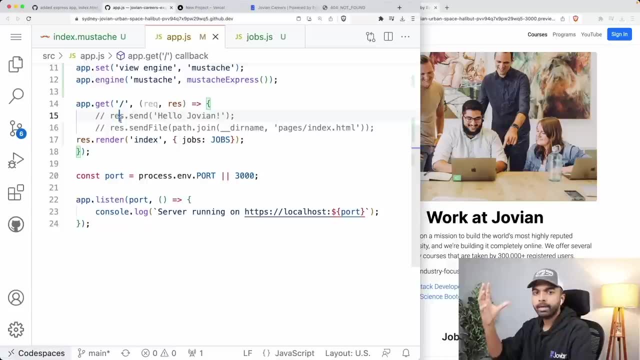 Okay, Now if you can wrap it, wrap your head around this, and you may need to just rewatch this a couple of times to get it- Then you've basically understood what most web servers do. They take some data from a database, put that into a template using some kind of a templating engine, and then they just send that data back to the client. 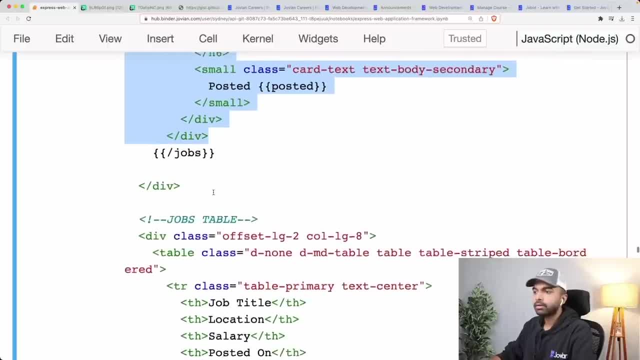 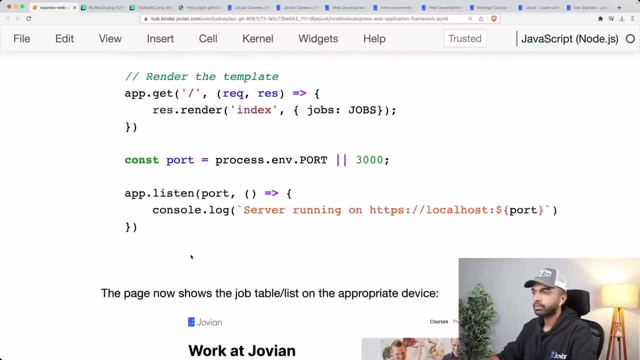 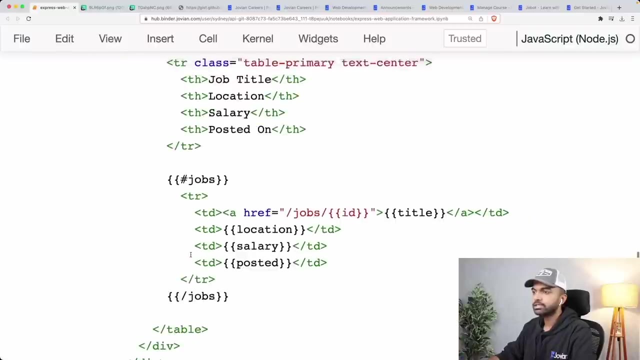 Okay, So that was the jobs Okay List, but why don't we also do the jobs table? So let me just grab the jobs table as well. Oops, Yeah, let's grab the. let's grab the jobs table as well. 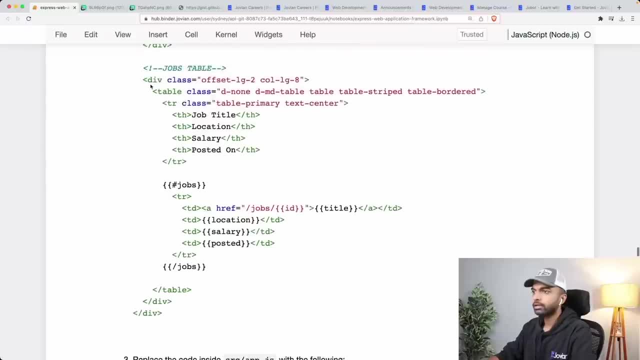 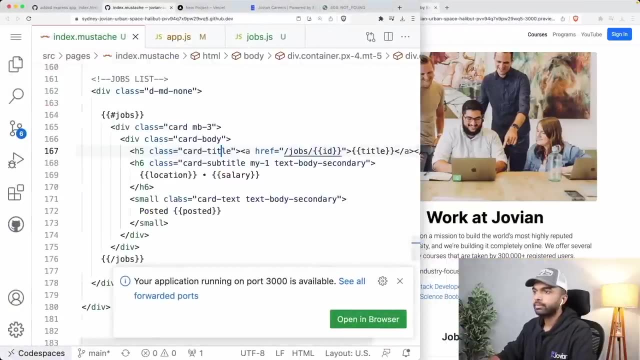 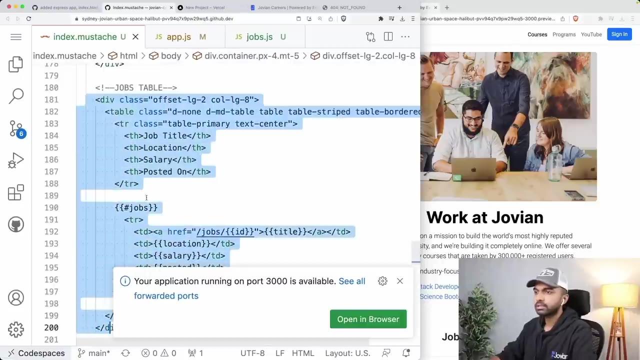 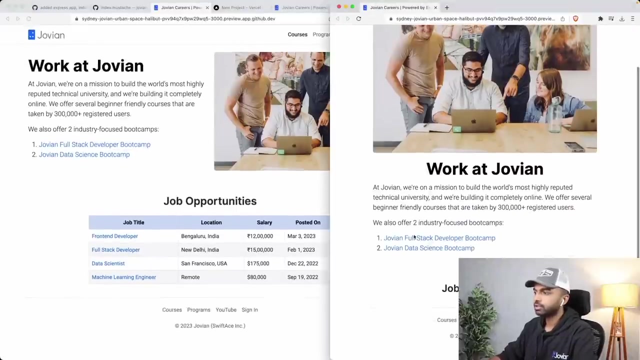 So I am going to zoom out here a little bit. grab this entire jobs table like that, and let's put that right below our jobs list. So that's our jobs table. Let me just give that a tab and all right, And now you can see that on mobile. I still have the jobs list. 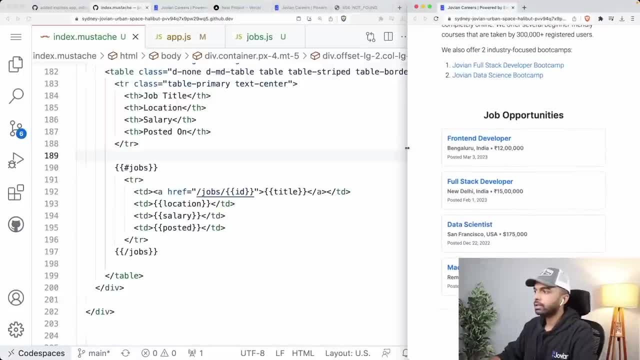 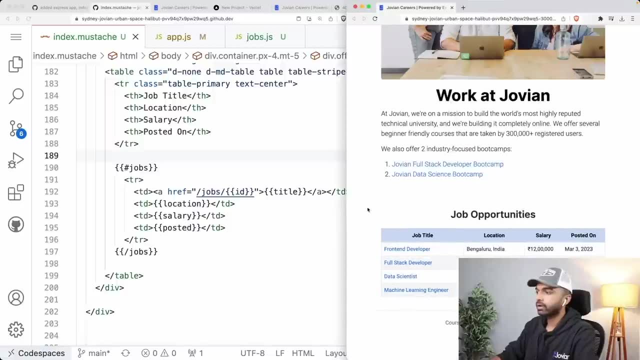 Yeah, On mobile I still have the jobs list, but on the desktop I have the jobs table. Okay, Jobs list on mobile. jobs table on desktop. How did we create the table? Again, we created a normal table with a table TR and it had a TH job title. 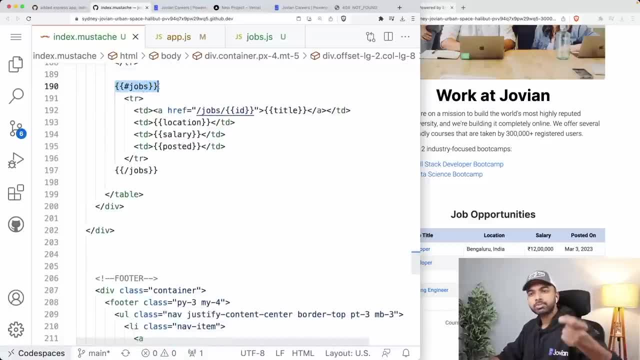 Okay, So that's our jobs table. Okay, So that's our jobs table. Okay, So that's our jobs table. Okay, But once again, we use the same jobs variable and now, using the jobs variable, we now created the title. 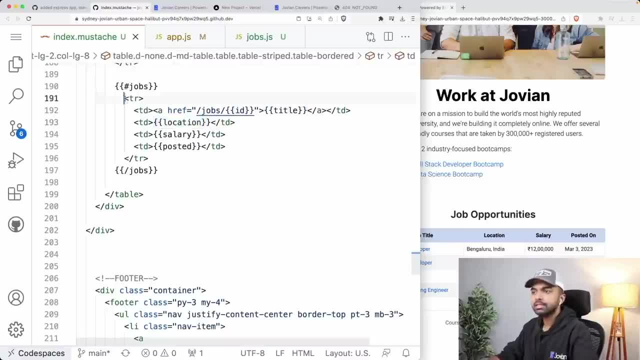 We created the location, we created salary and posted that, And we, this time, we created not a card, but we created a table row, and four of these rows get created And each of them is going to have the appropriate information. Okay, 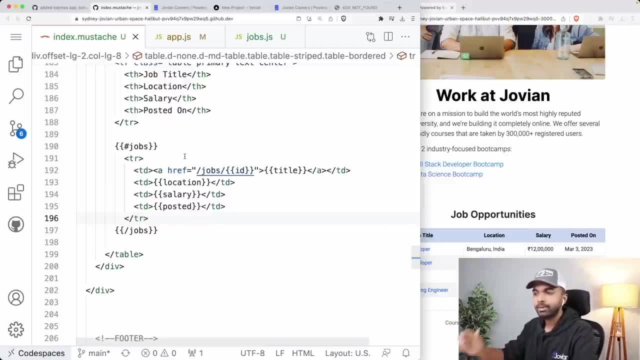 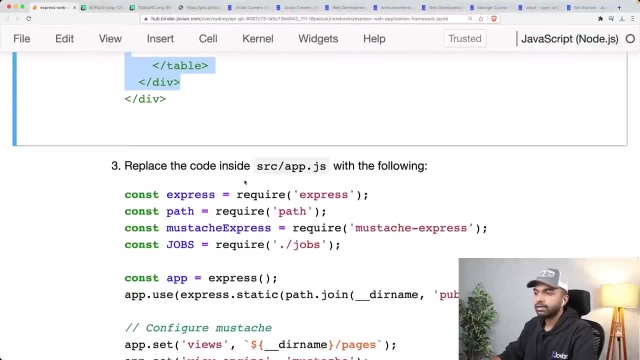 So just understanding this templating syntax can sometimes be a bit tricky at the beginning, but once you get it it becomes second nature And mustache is actually really simple to understand. So with that we have rendered The mustache template You can see. here we say rest or render. 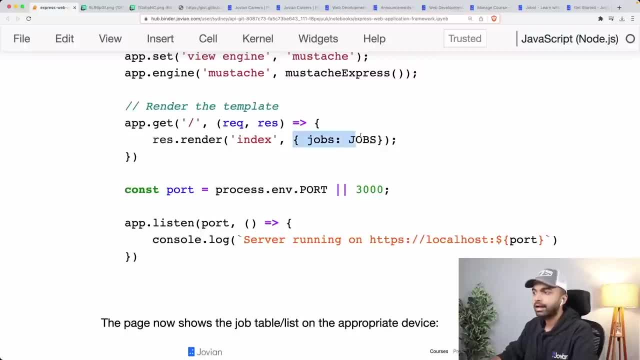 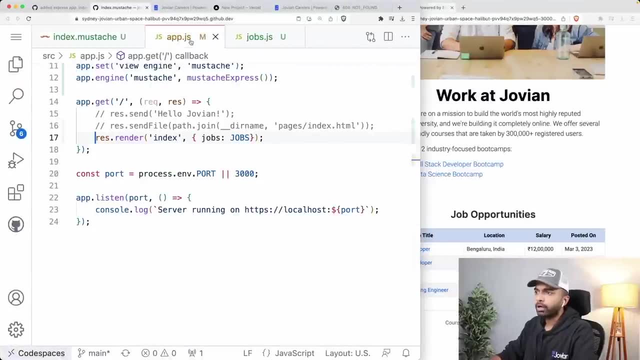 We've given it. we've given it the name of the template, index or mustache- and a list of parameters that we wanted to pass in. Okay, Now, of course, if you wanted, we could also pass in more parameters. For example, I could pass in a parameter called company name and I could pass that. 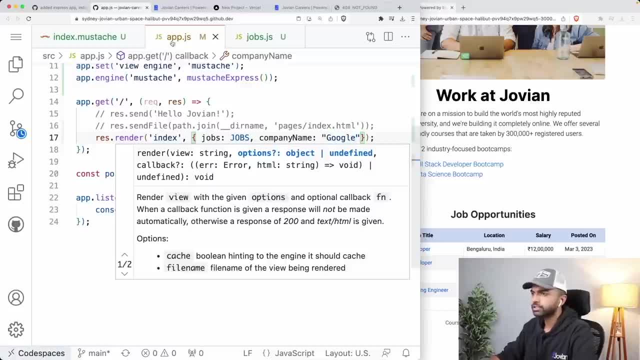 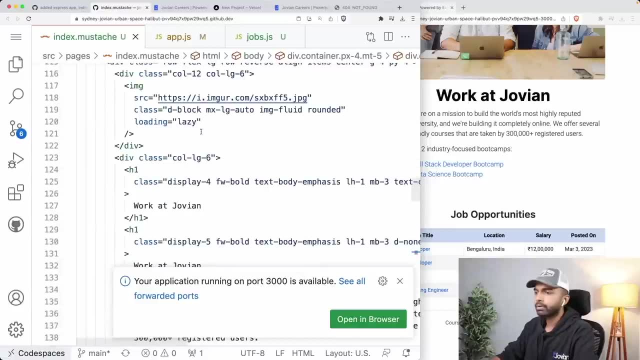 in as, let's say, Google for just, for example. then in my index or mustache, I could come in here, right at the top, where I have my age one. where is that? Yeah, So I have, I have my age one. and here, instead of saying: work at Jovian, uh, I. 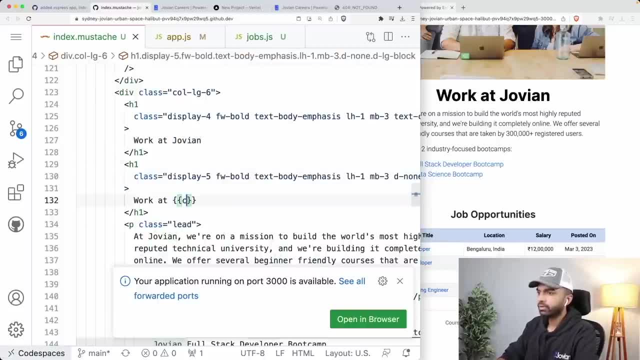 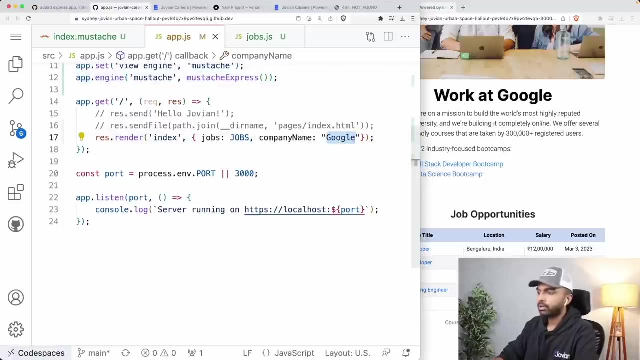 could maybe have just done work at company name, all right. And if I had done that work at company name, you would see that now it would say work at Google. So you can pass not just one parameter, but you can pass any. 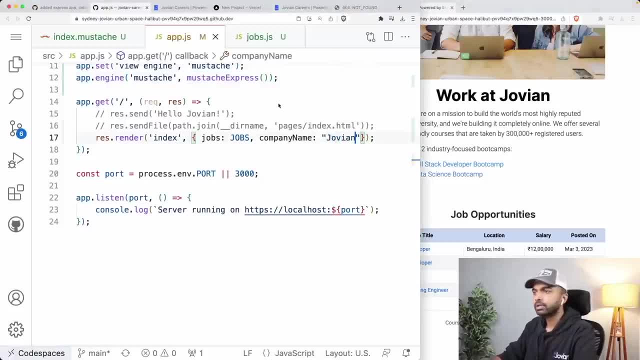 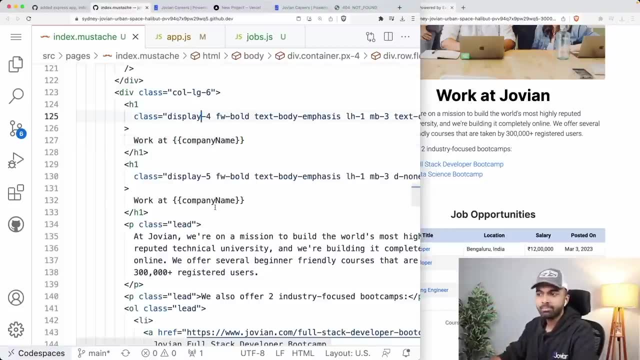 number of parameters you want. And now I'm changing Back to Jovian and it says: work at Jovian and you can modify any part of your template as you want. You can modify something inside the class, inside the tag name, whatever you want. 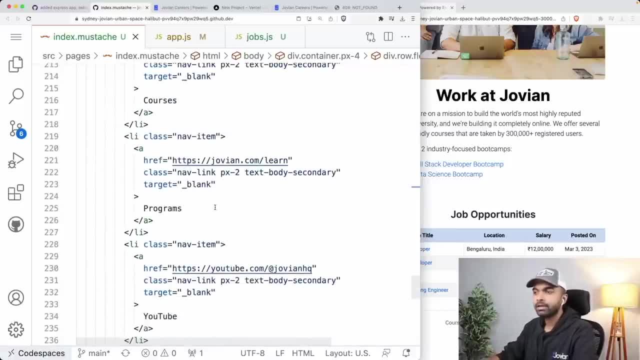 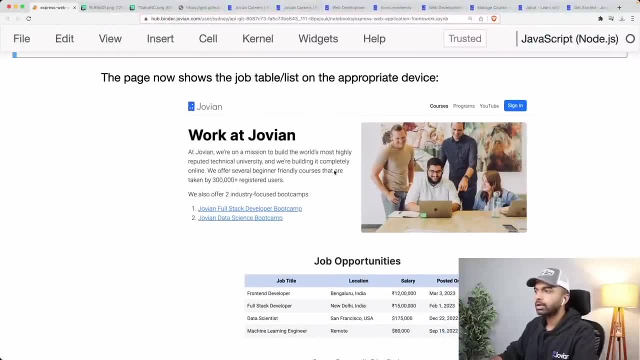 The templates are very flexible, but also they can also be a little tricky to work with. for the same reason. All right, So now the job. now the page shows a job table or list on the appropriate device. So now it says work at Jovian, and now we have the job opportunities table. 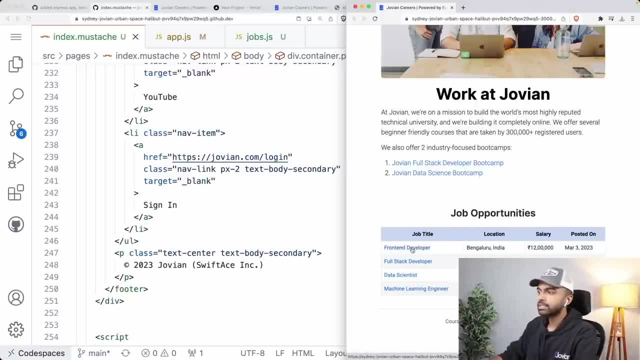 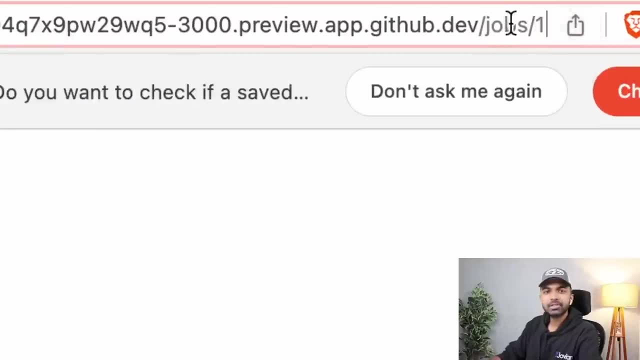 One thing I want to mention is we have also added links to these tables. So what happens is when you Click this link, it goes to this: If you, if you see here at the end of the URL, it goes to slash, job, slash. 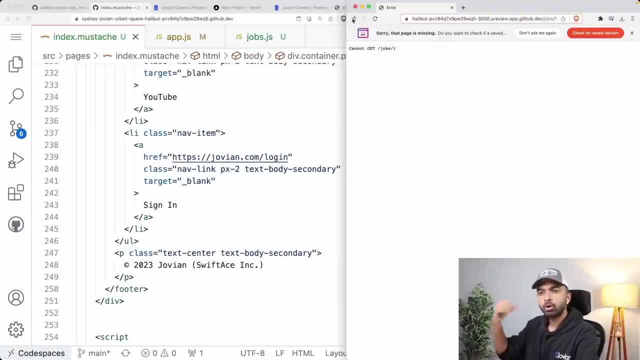 one or two or three or four, based on the job ID, it's going to go to a different route. So the next step for us is going to be implement that route page, implement the individual job pages for each of the jobs, and we'll see how to do that. 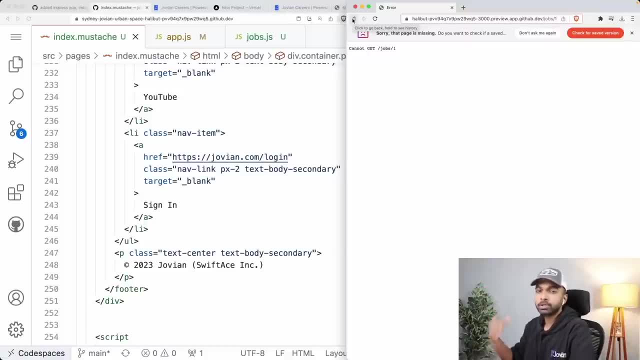 in a dynamic fashion, once again without having to create four separate pages, because you could have a hundred jobs or you could have 50 jobs. So you do not want to create a hard code the number of jobs you have. a Create a bunch of routes anticipating how many jobs you'll have. 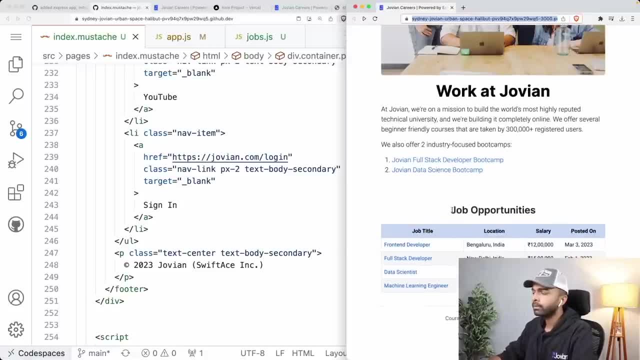 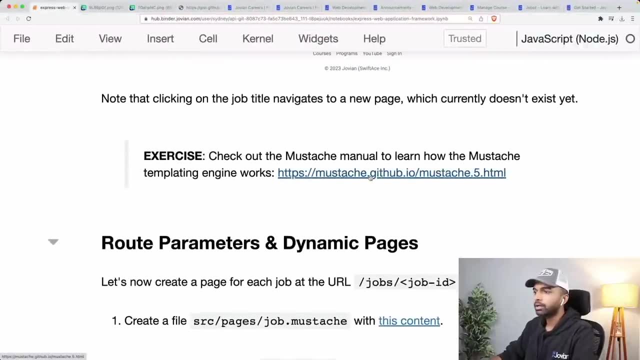 You should just be able to handle any number of jobs. Okay, So that is our second step, And I would encourage you to maybe check out the mustache manual to learn how the mustache templating engine works. It's actually really simple. 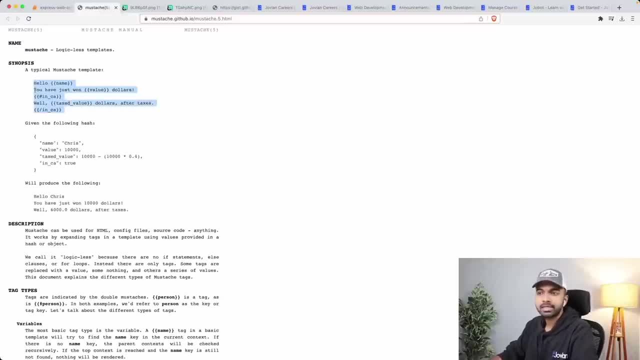 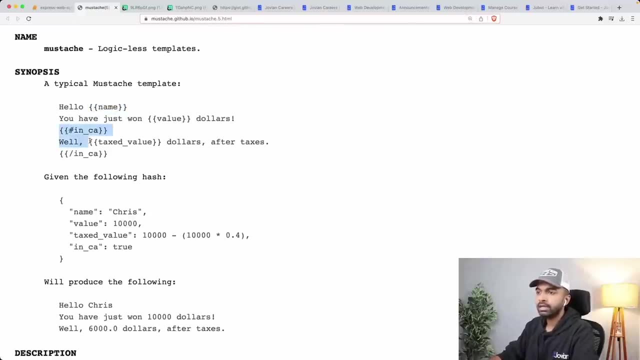 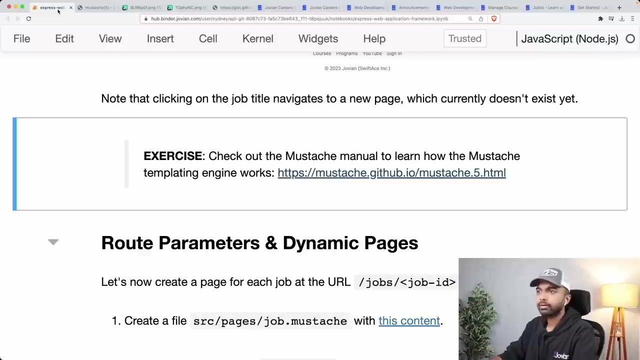 All it does is, given some texts like this- it could be HTML CSS, whatever it- and given a bunch of these template tags, name value in and slash in or whatever it can, So you can take this data and it can just simply fill that data into this template. 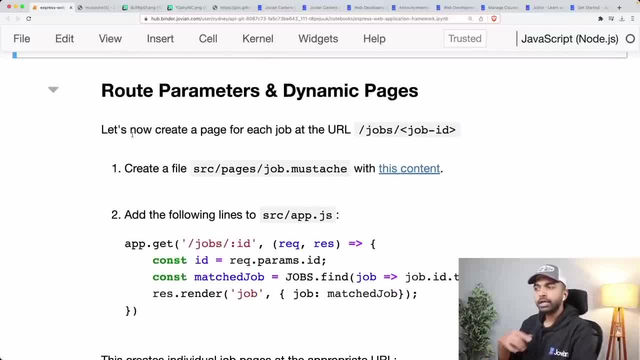 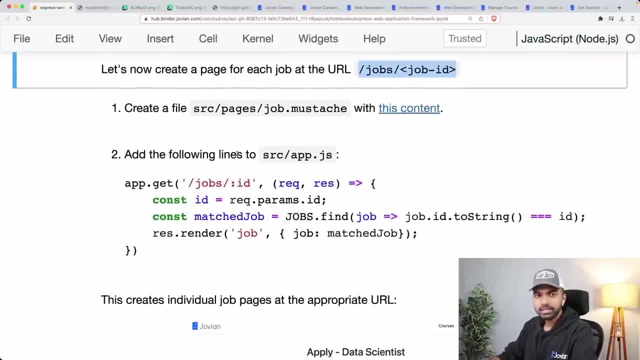 Okay. Now the next step for us is to create a page for each job at the URL: slash job, slash job ID. Okay, And But this we are going to again follow a two-step process. First, we're going to create a template for that particular job. 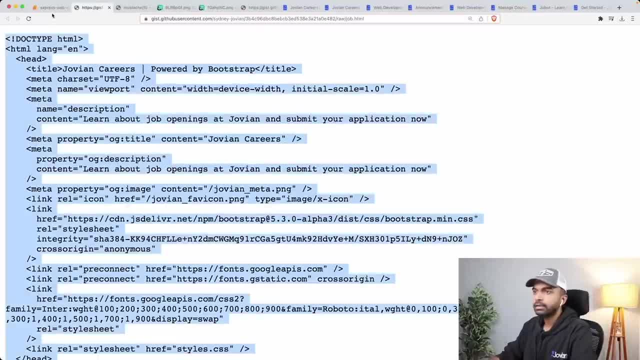 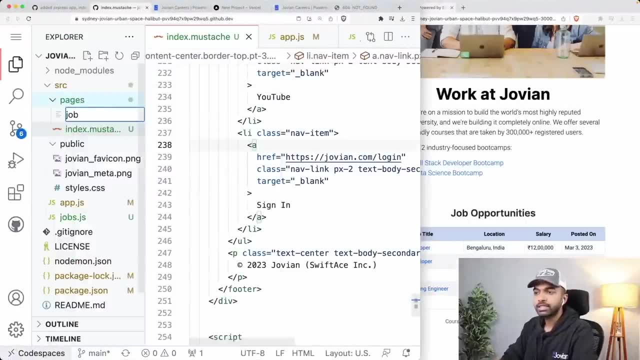 So I've already again put together some content. So I'm just going to create another template. It's called job dot mustache. So in the pages file I'm going to go in the pages folder I'm going to create job dot M U S, T, S, C H E, job dot mustache and let's close. 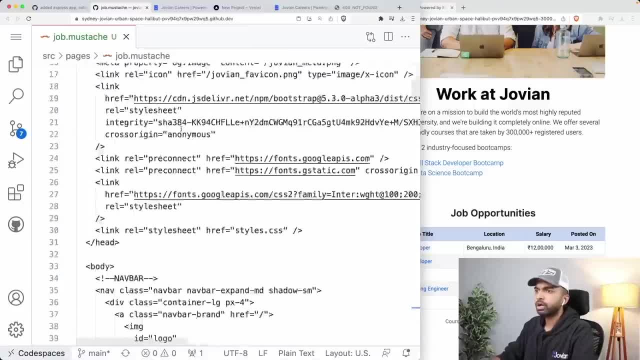 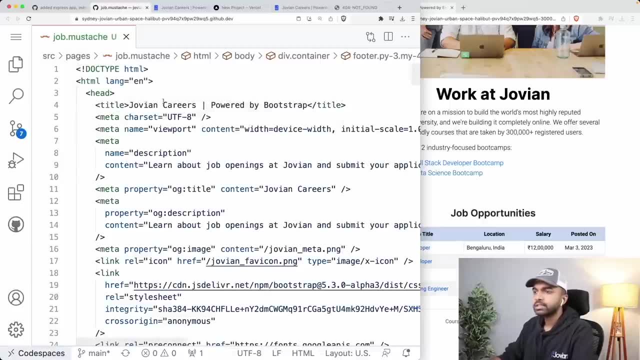 everything else and let's paste in here the job dot mustache file, And what does it contain? Well, let me just change this formatting to HTML. Yeah, So what does this contain? This contains again a bunch a head, basically a bunch of meta tags, et cetera. 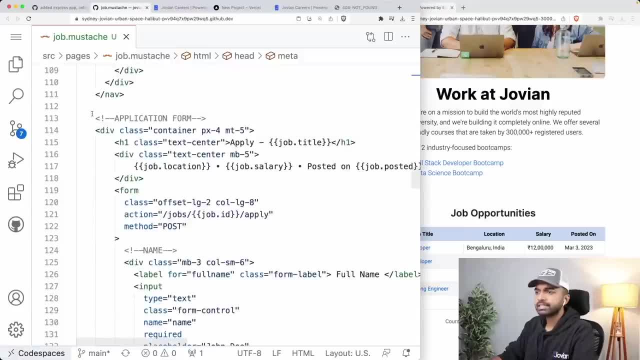 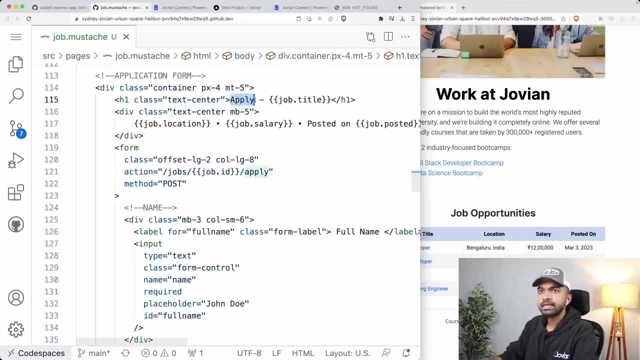 Then it contains a body. in the body It contains the nav bar. So it's the exact same nav bar that we have in index or HTML. but then it contains an application form. Okay, So it contains an application form, and here it says there is an H one that says: 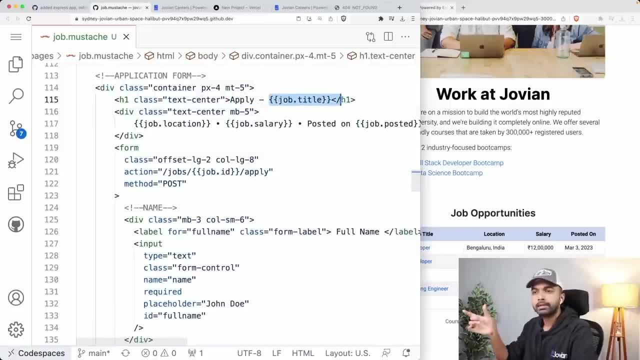 that it is going. it is going to say apply job dot title. So you can already guess here that it expects to maybe get a variable called job which has a title field inside it or a title key inside it. Similarly, it expects to get the variable or input job which contains a location. 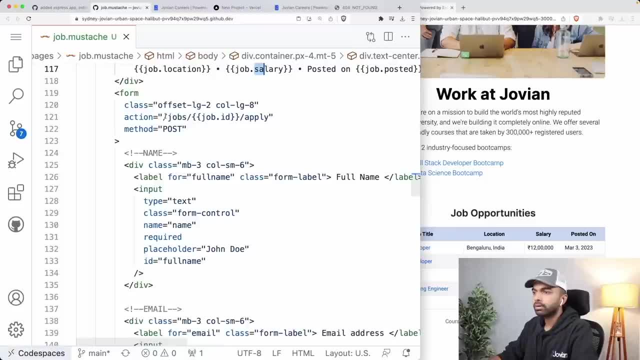 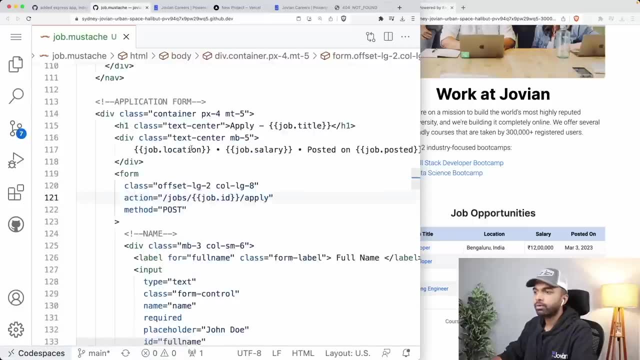 and a salary and a posted information, And also it's going to Create this form, and the form action now is also going to be something different- We'll come and touch on this later- but then it renders this form over here, this application form, and then it renders the footer below it. 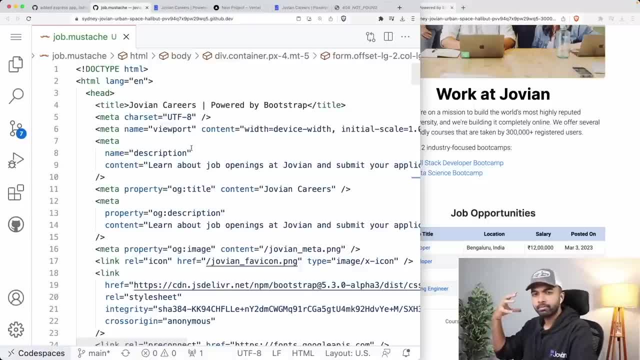 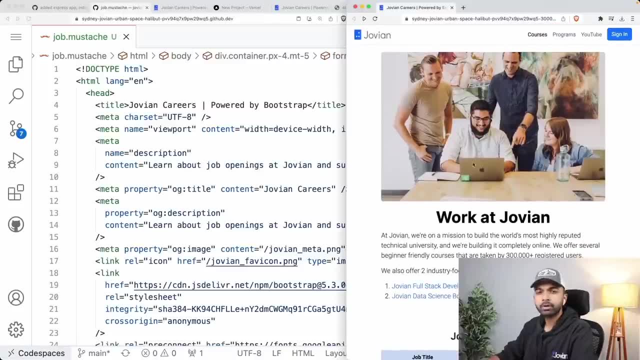 Okay, There's. no, yeah, there is a footer here as well. Okay, So we have. you can already visualize that this is going to render the same page, but instead of the about section and instead of the table, it's simply going to show an. 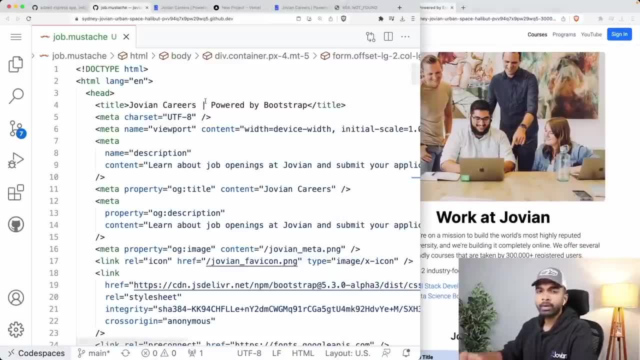 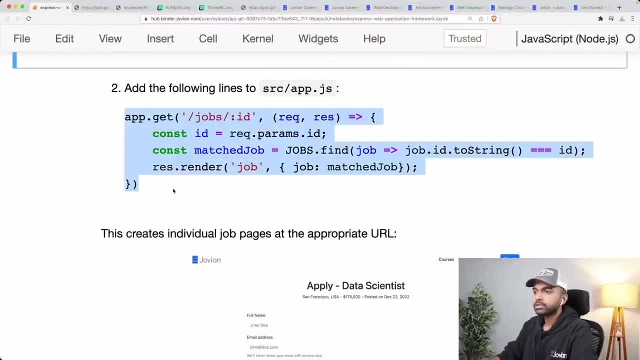 application form with a title on it. Okay, But how do we actually show this page when you try to access a job? that's where? Okay, we now need to add a new route. So here's the route that we're going to add. 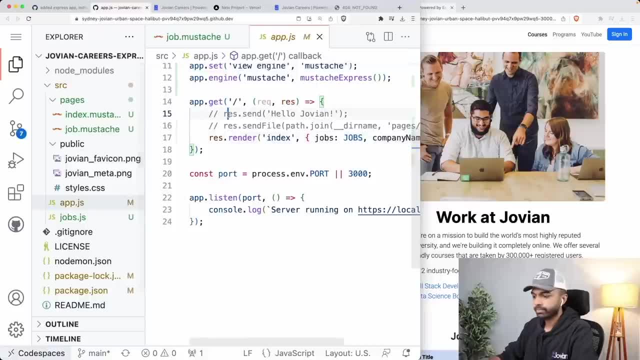 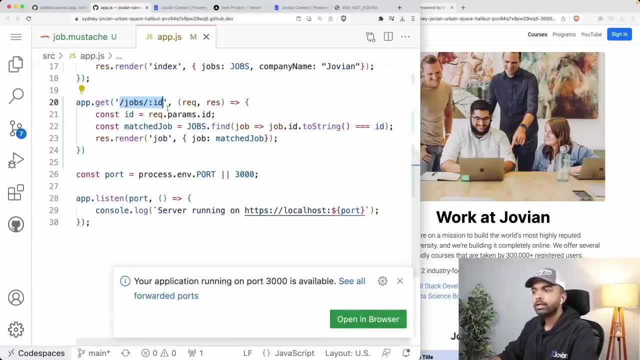 We are going to go back into appjs, And now we're going to create a new route. This time we're going to say: appget, slash jobs, colon ID And in this case- and you see here we've not put in a particular job ID- 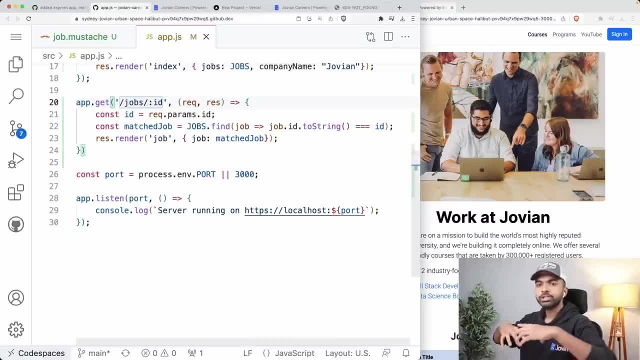 We could have put in: slash one, slash two, slash three, slash four, but we have created a more generic route and this is called a route parameter. We've created a more generic route that can handle anything After slash job, So it can handle slash job, slash one, slash of slash two, slash of slash 99, slash. 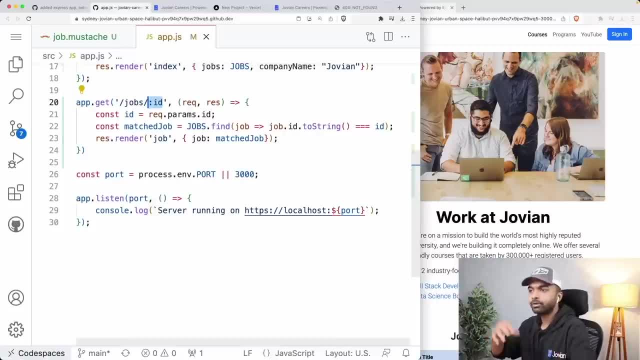 job slash, hello, slash job slash by slash job slash. Google. It could handle anything, but of course we want to maybe do some filtering and ensure that it's actually a number, a job ID, Okay, So what we do then in our route handler function is we get the ID. 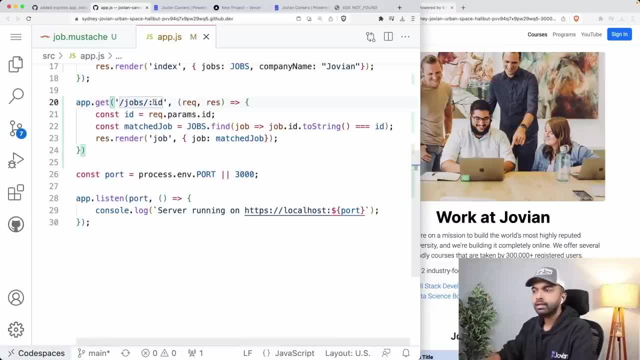 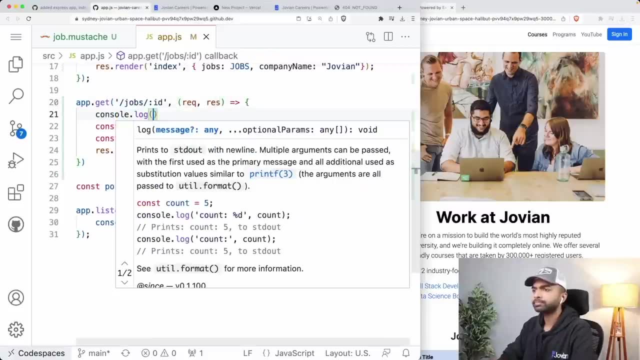 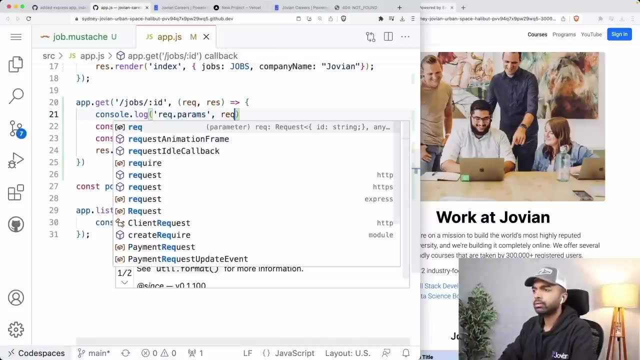 So whatever is indicated using a colon at the beginning, you can access its value in request dot params. Okay, You can always just go in here and also do console dot Log, rec dot params and that's going to print reg dot params. 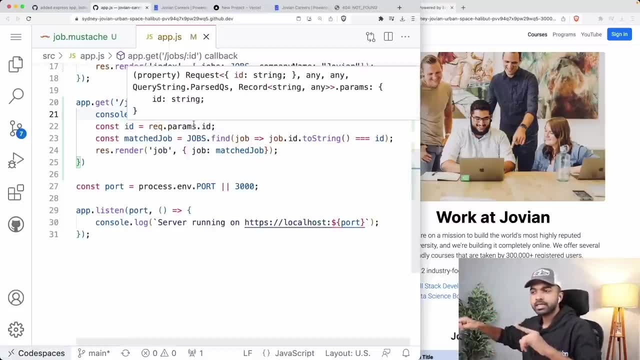 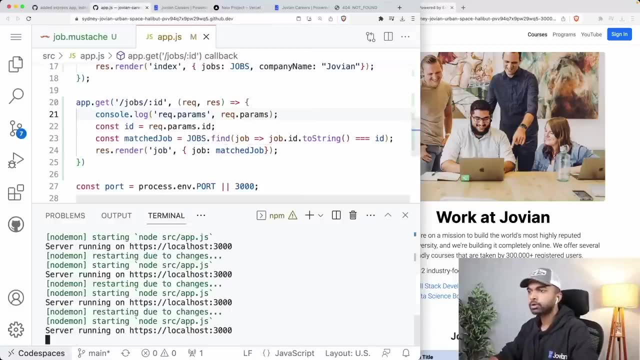 Okay, And, by the way, this console log is not going to show up on the browser. This is actually going to show up on our terminal down in the server over here. Oops, Yeah, this is all. this is going to show up in the terminal. 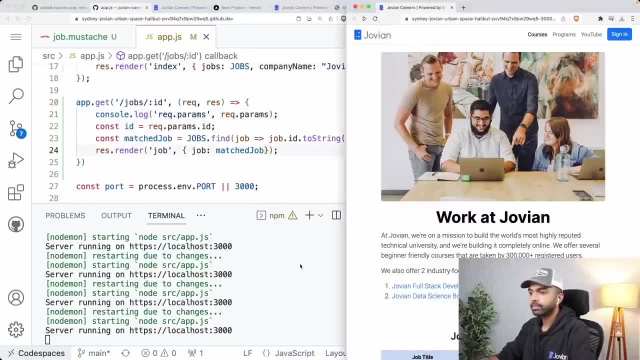 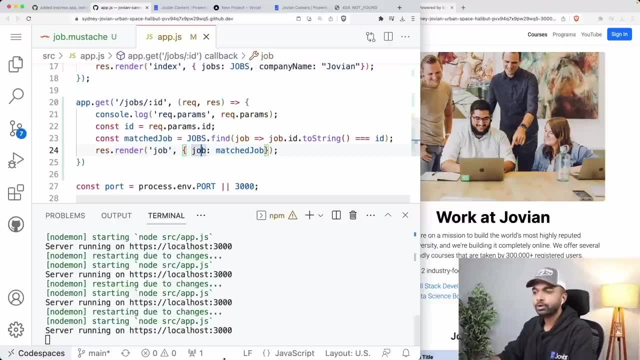 down in the server over here. So if I just run the page once again and open that, and if I actually try to open that particular page, that, uh, that particular route, then it is going to show up here in the server. 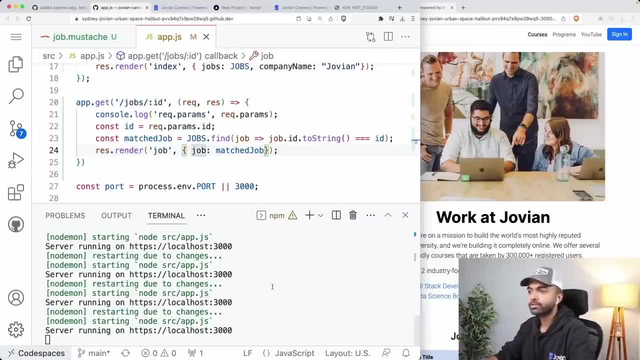 It's not going to show up in the browser. So remember what is executed on the server and what's on the browser. All right, So we get the ID that is present in the route parameter and then we try to find. so we are using the find method of an array. 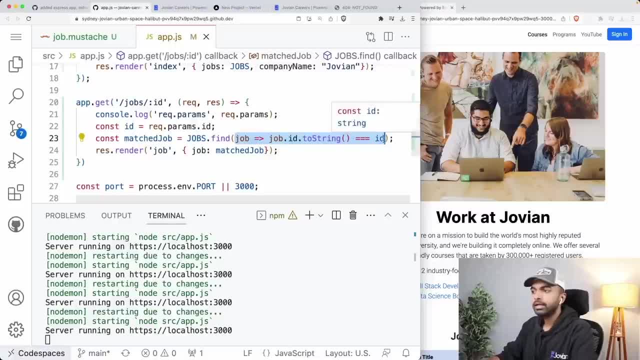 All it does is given a condition or given a function. it finds that job, uh that element which matches that condition. So we are saying: jobs dot find, given a job, the job dot. ID dot two string. So we've done two string here, because the IDs here are numbers. 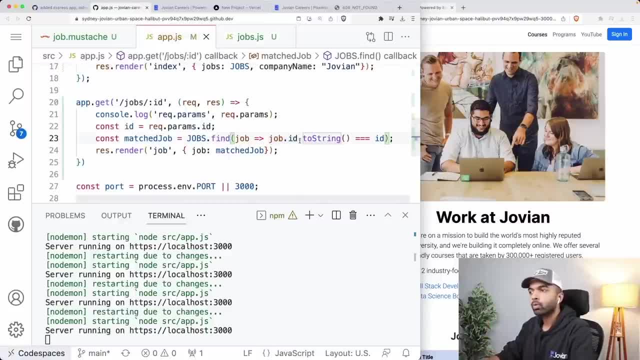 So what we're saying is: in the jobs list, find the job whose ID, when converted to string, matches the ID that we got from the URL. So from the URL we get an ID and we search for the job matching that ID in the jobs. 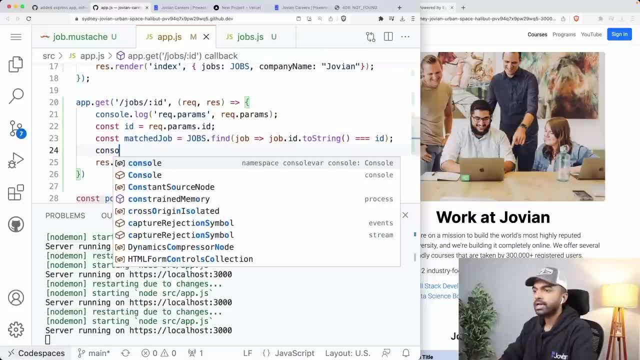 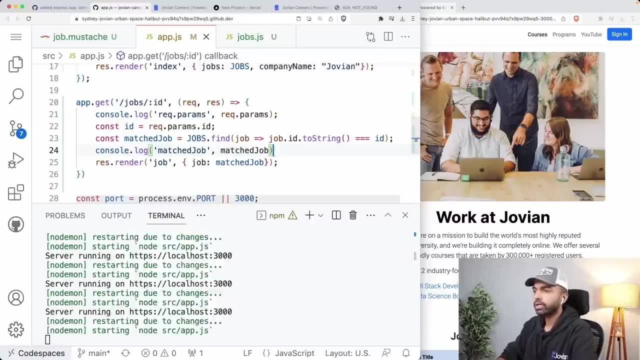 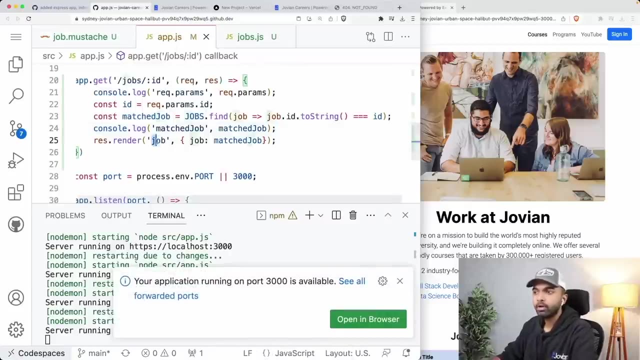 table and that gives us a match job And let us also log the matched job. So console dot log matched job and let's log match job, Okay. And finally we are saying Rest dot render job. So we are, we are rendering the template job dot mustache this time, which is: 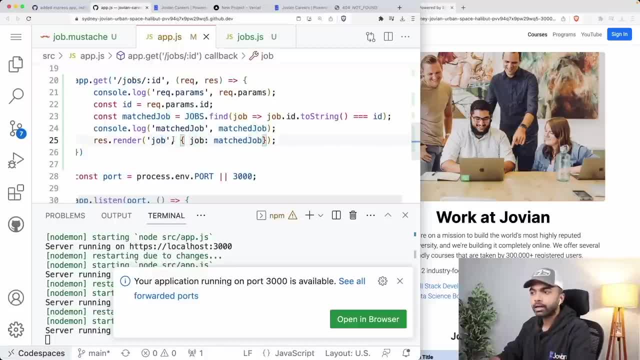 present in the pages folder, which is configured as the views uh for our express. so we are rendering the job dot mustache template and we are rendering it with the data job, where the key job or the variable job will have the value. 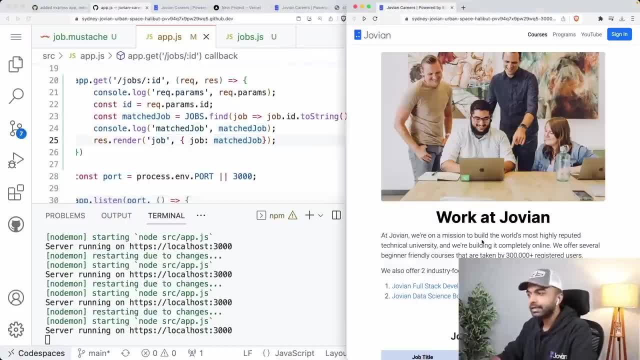 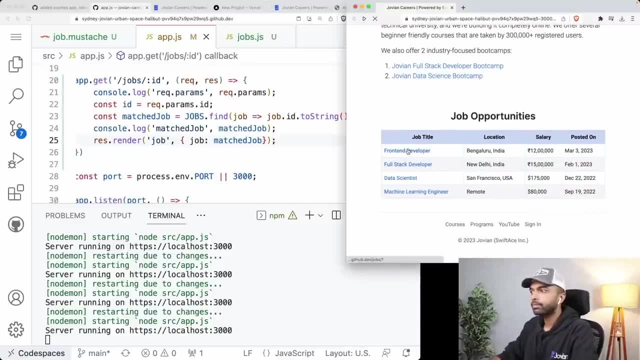 of match job. Okay, So let's just run this. Let's see it in action and things will become clearer. Let me click on front end developer over here. Yeah, Let's click on front end developer And you can see now, magically, we have navigated to slash job. slash one because 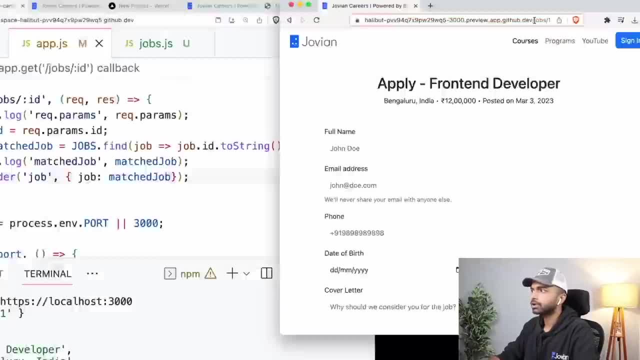 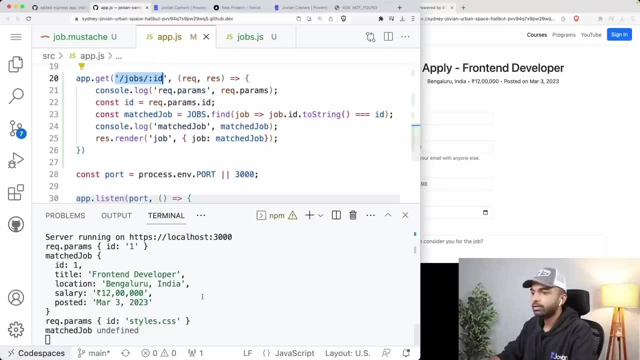 that is something that we configured in our index dot JS template. We've navigated to slash job, slash one, So that automatically gets caught by this route handler And when it gets this ID, you can see that the ID printed here is one and. 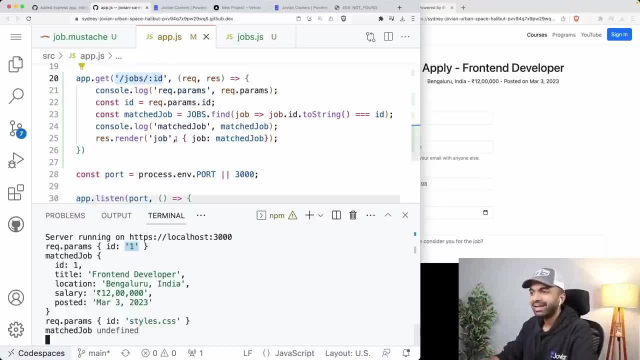 you can see that it's a string. So by default all route parameters are strings And then we try to search for that ID within the jobs area And we got back a match job. and this was a match job. It had the ID. one title: front end. 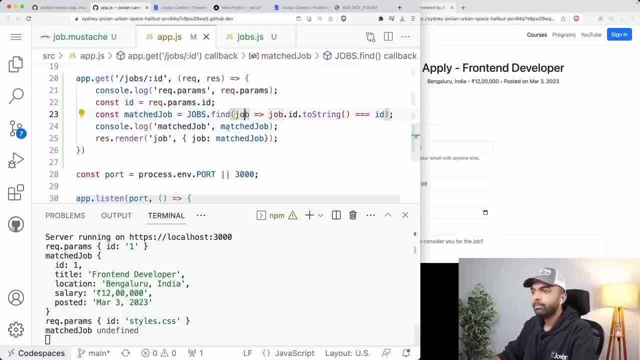 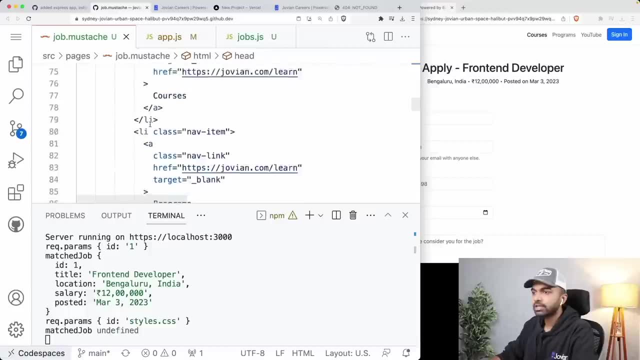 The job was match developer location, Bengaluru, India, salary, et cetera. And then we put that into the, into the template like this: And in the template job dot mustache. we are actually using it to render things. So we are using it to render the job title which is showing up here after apply. 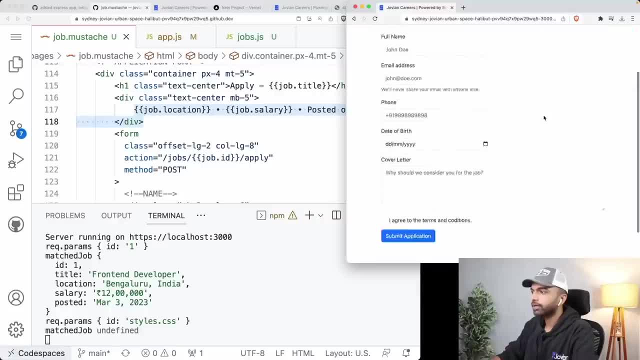 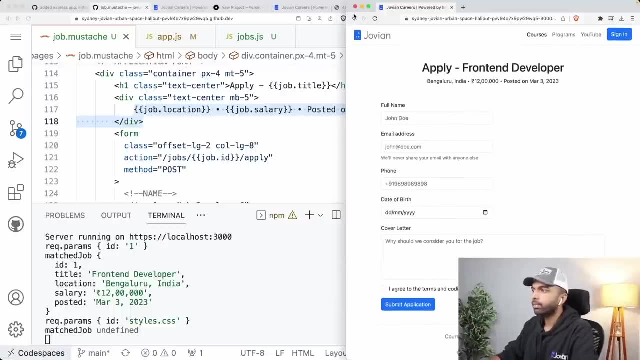 We are using it to render the job location, job salary and posted on, which is all showing up here, And the application form is generic. There is no change here, So that's I think that's pretty neat. Now we can go back. 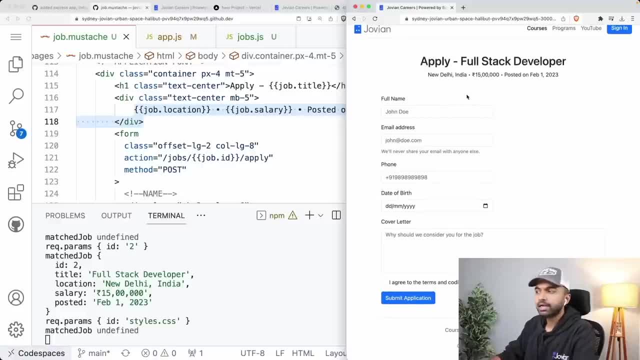 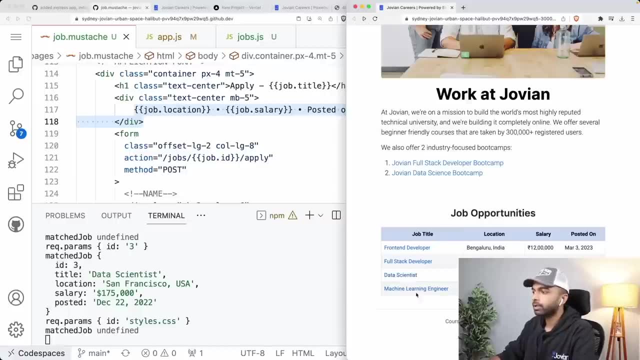 Okay, Let me open: open full stack developer, And now it says apply full stack developer And there's a different salary and location. Let me open data scientist, Now it says something different. And let me open machine learning engineer, And now it says something different. All right. 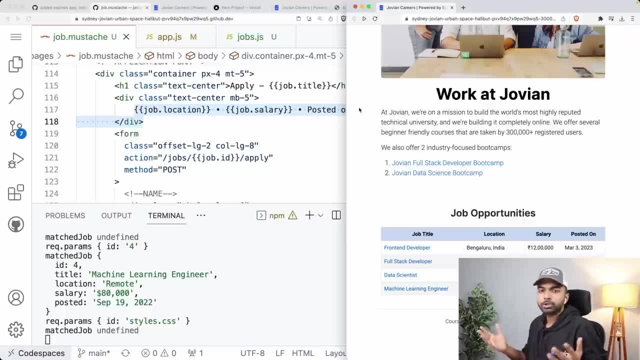 So that way, with just one route, we have handled four jobs, but not just four jobs, potentially hundreds of 1000s of jobs. on Jovian, For example, we have hundreds of 1000s of notebooks that people have created, But there is only one route that is serving every notebook right. 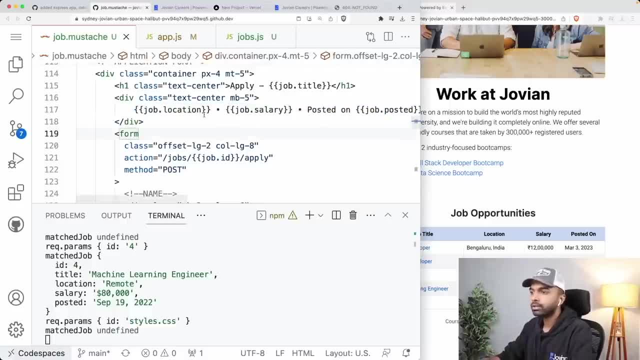 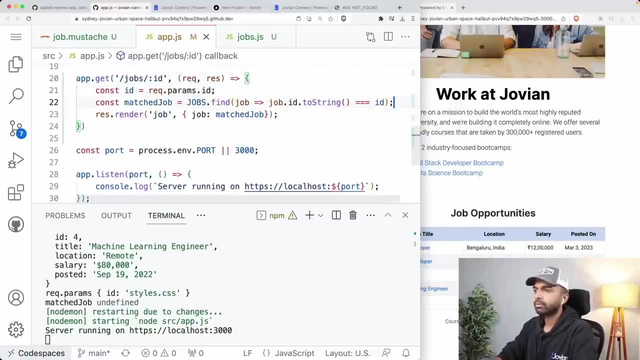 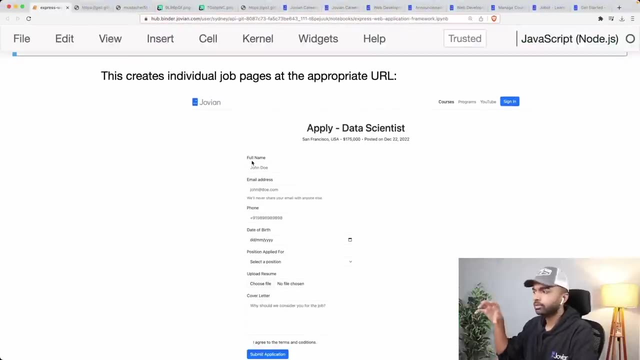 And that is the benefit of having web servers and web applications that can do all this kind of dynamic stuff. Okay, so let me get rid of these console dot logs And now we are ready to move forward, because now we've created the single individual job page. So 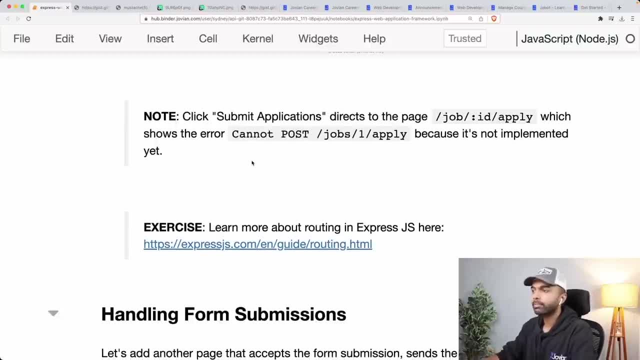 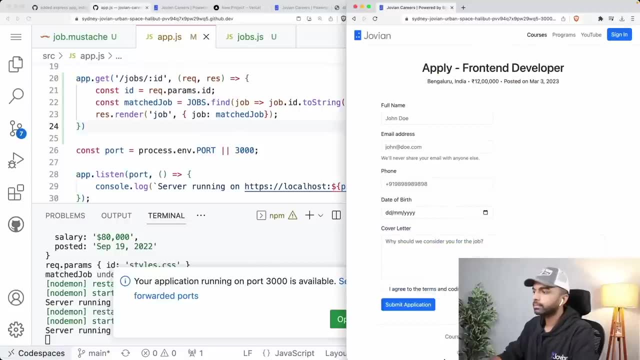 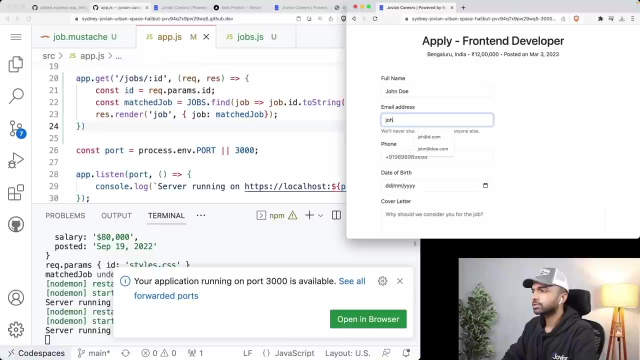 the next step for us is going to actually support submitting the application. So if you see here, if I click on a job role and I fill out the application- let's say I fill out John Doe and I fill out the email address john at doorcom And 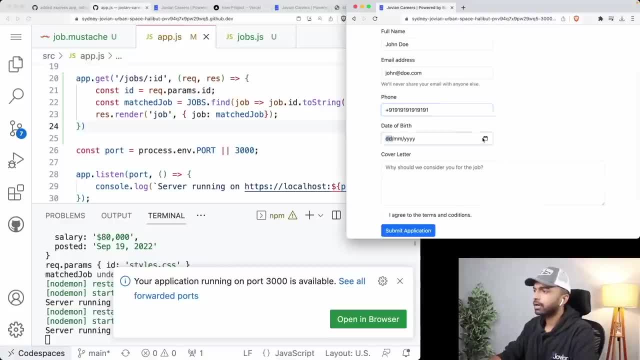 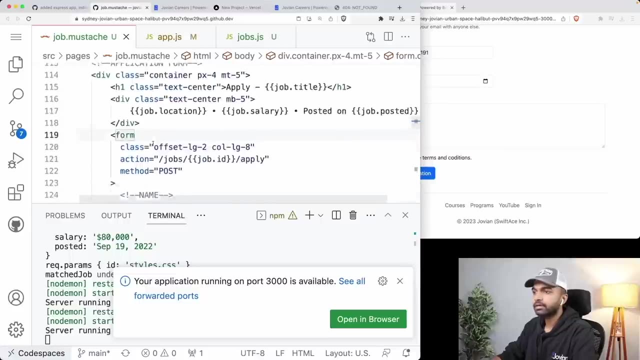 I fill out a phone number And let me fill out a date of birth here, And we fill out a cover letter And agree to the terms and conditions, click Submit application. So now what happens when we click Submit applications is, in the form we have specified, a certain 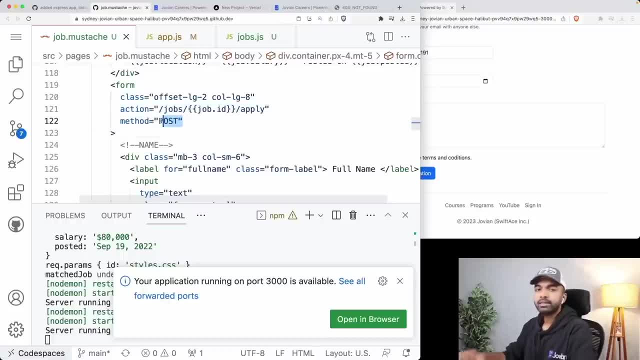 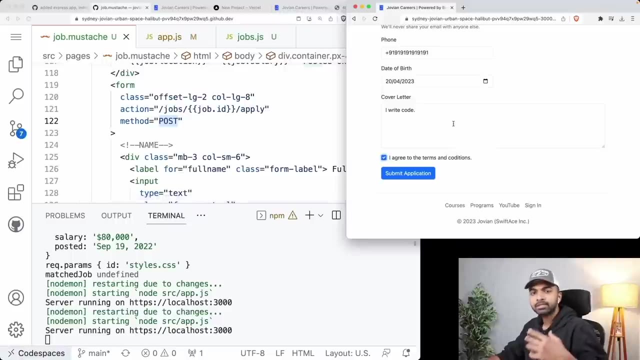 action. So, and we have specified a certain method, So all of this data is going to be posted. So there are two ways, two methods we can specify. one is get, one is post, And I'll talk about the differences as well. get simply means that all of the parameters or all of the data that 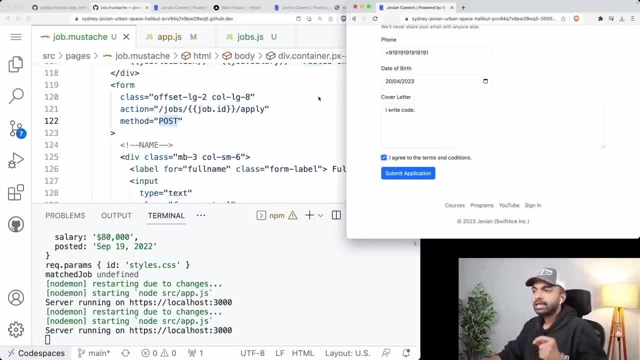 has been filled in into the form will be sent as part of the URL, Whereas post means that the URL is going to be just this: the data that is there in the form is going to be sent as the body of the request. Okay, so every request has a URL. 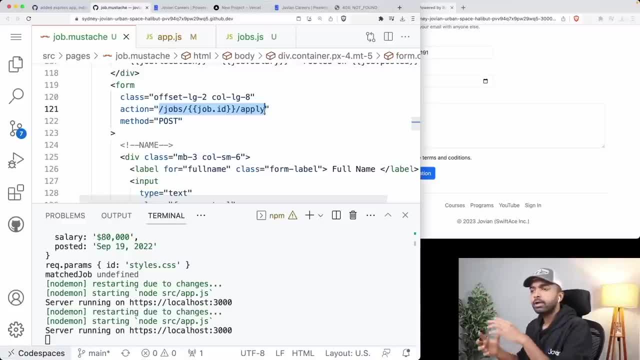 And a body and it has something called headers as well, which we'll talk about later. But a URL in a body get is going to just put everything in the URL. your URL is going to become really long with your cover letter and name and email and everything which is something we may. 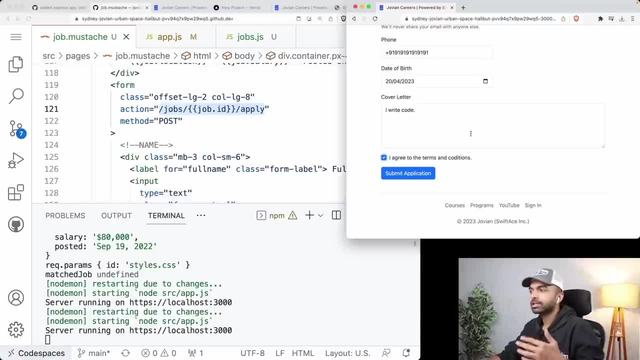 want to avoid, especially, if you can, if you have these text fields with a lot of content. So that's where we use post. So in post this, we are simply going to send this data to this particular URL: slash jobs slash. particular job ID. slash. apply on the server, But we're 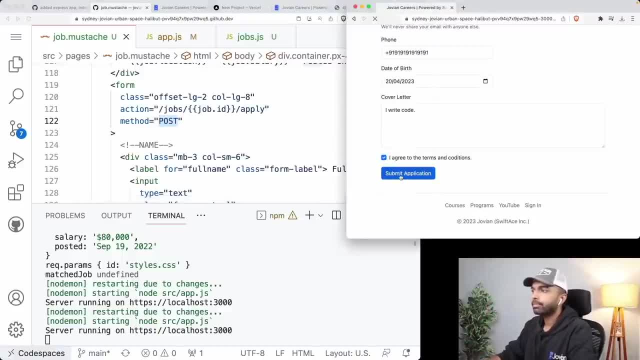 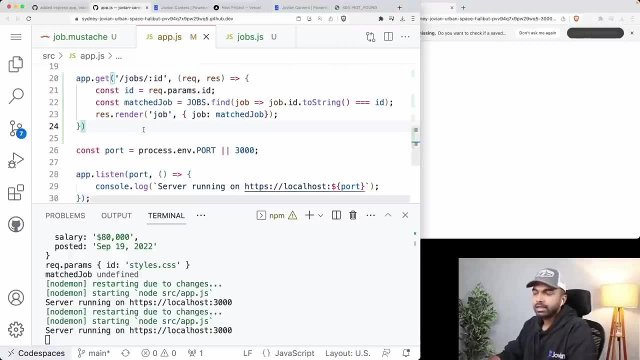 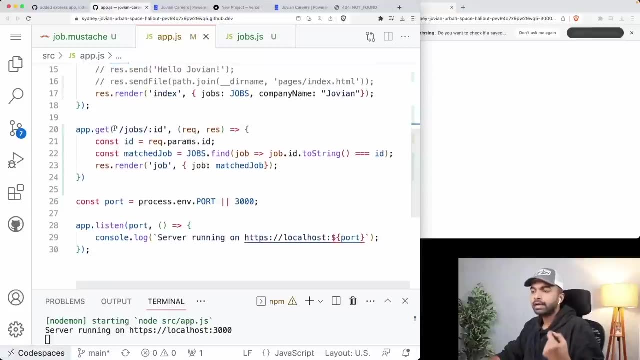 going to include all the data in the request body And let me click Submit application And it says cannot post slash jobs, slash one, slash apply. Well, that is because in our web server currently we can only, we've only handled the slash route and we've only handled the slash job, slash ID route. Well, we could. 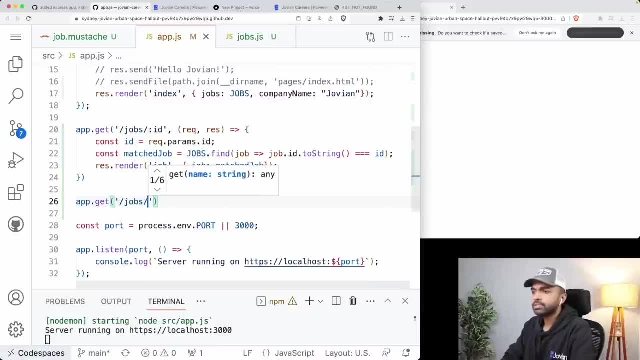 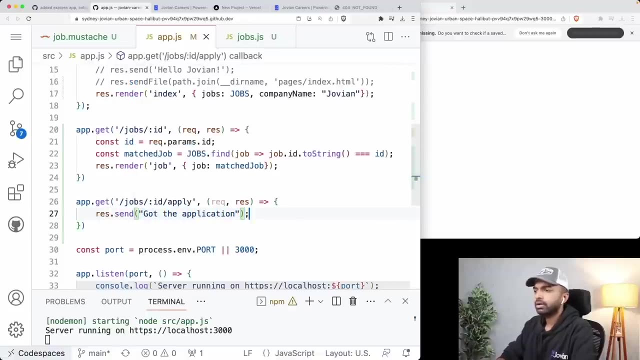 try to handle it like this: we could say: app dot get slash jobs, slash colon ID, slash apply. And we could say something along the lines of rec res And let's say let's simply send rest dot send, Got the application. Let's see if that works. 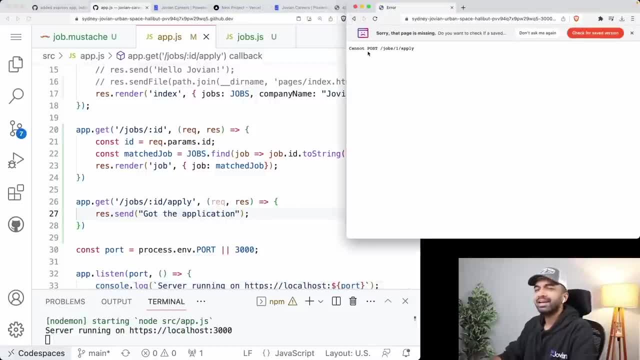 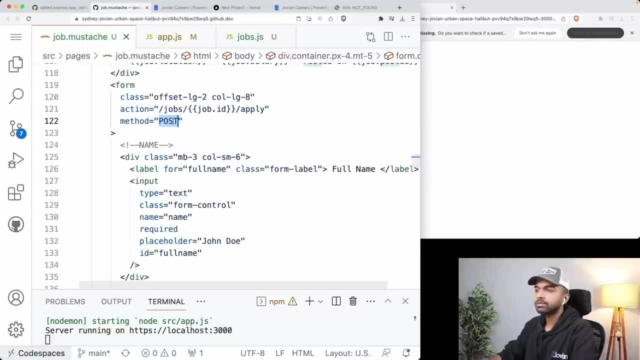 So let me go back here And let me click Submit application, It still says cannot post. That is because here I'm listening for the get HTTP method. So if I was sending the data using the get method like this, then it would work. So if I click Send, I'd have to reload. 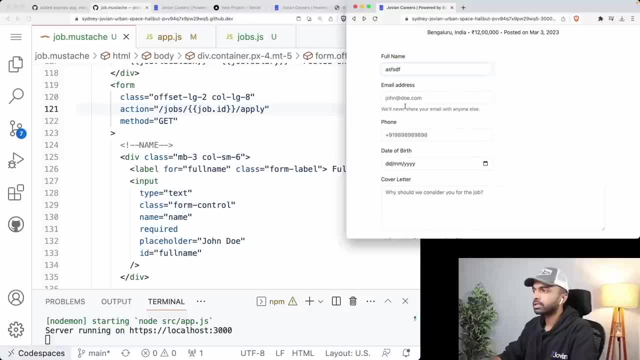 the page. Yeah, so if I just put in something here, a at bcom, And if I click send, I'd have to reload the page. Yeah, so if I just put in something here, a at bcom, And if I click send, I'd have to. 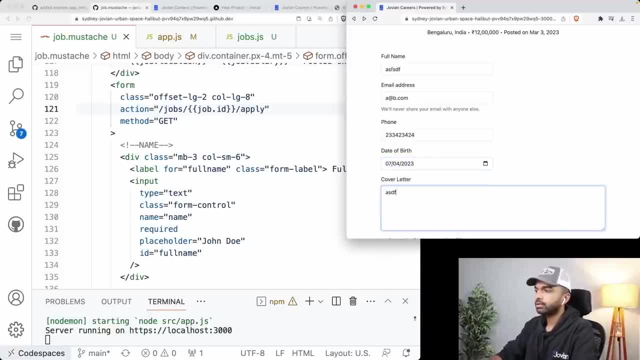 reload the page. So if I just put in something here, a at bcom, And if I click send get, most I'd have to import something here, a at bcom, And if I click send get, I'd have to import something here and something here And something here And I click Submit application. Now 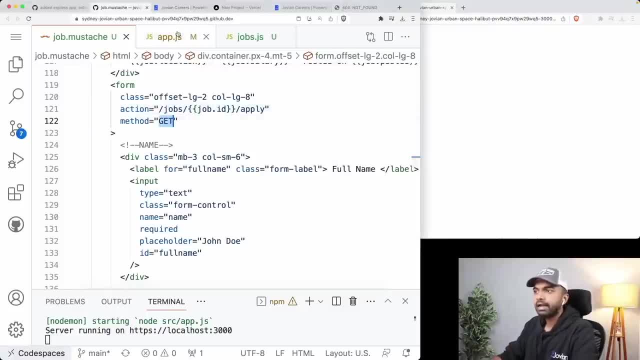 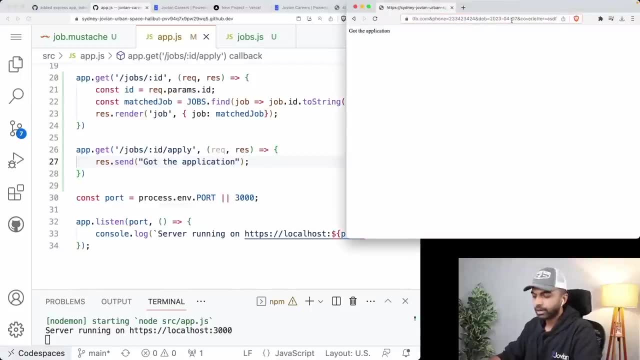 it says got the application. So when I send with the method get and I have a listener with the method get, it gets the data. but where does the data? all of that data is here, right here you can see it's part of the URL. 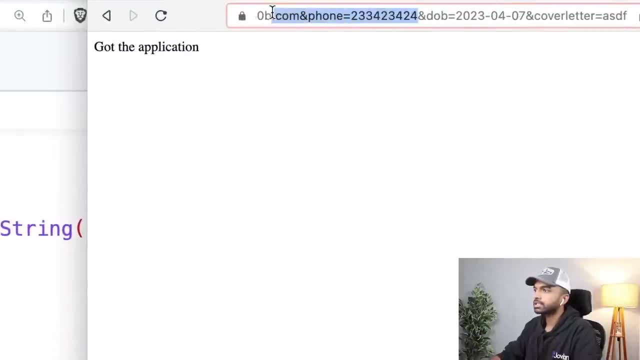 It's all part of the URL. foreign equals such and such, email equals sagan searchcom, And name equals sudden search, And this is not a good idea for long, for longer form. So short, pro short format. Now it's totally up to you. brows or files to us If you don't know either. 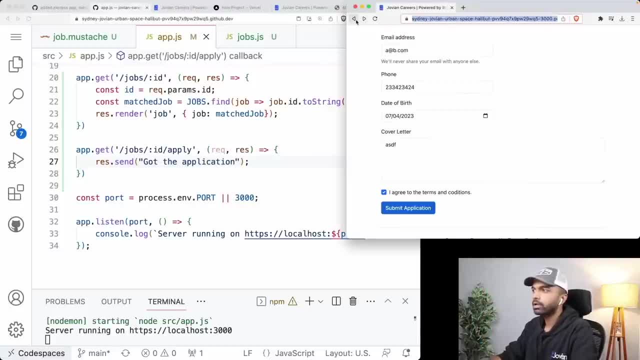 long, longer forms. for short forms It's okay, But for long forms it's not good. But on the other hand, what we want to do is we actually want to send it with the method post and we want to listen to it with the method post as well. Okay, So this time, when I reload, 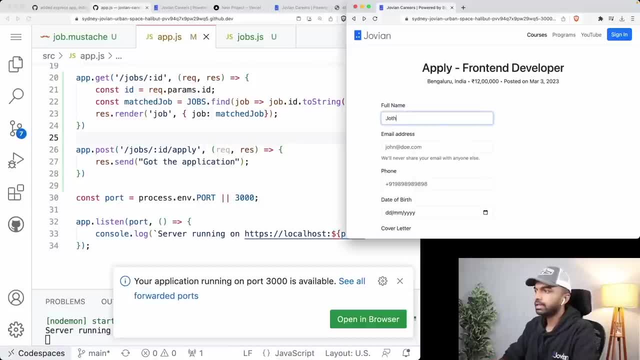 this, and let me pull that in again: John Doe a date and something and submit. Okay, Doe at ecom and submit. this time You can see that we actually listened. So every request and hence every route, has two things. It of course has the route. 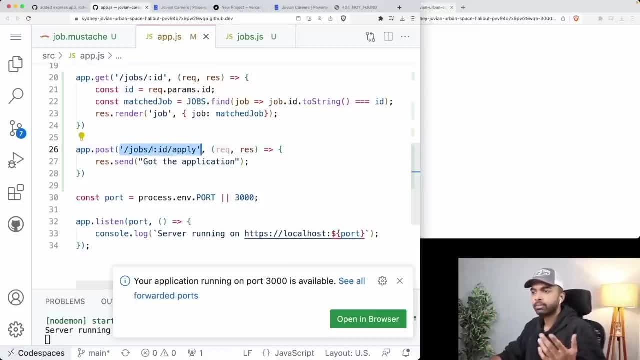 Which is going to match the specific route, depending on the parameters, and it has a method. So we need to do accept form submissions which are sent using the post method. We need a route that can that is declared using the post method. Okay, And now here we will be. 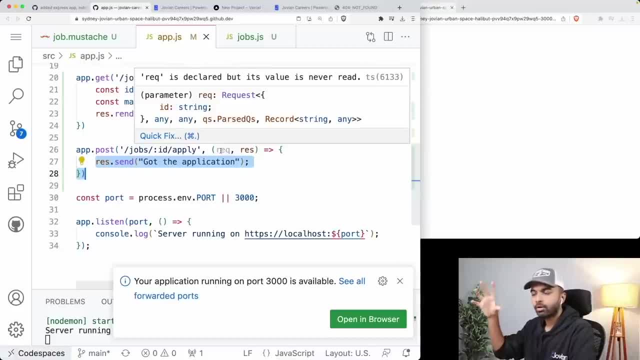 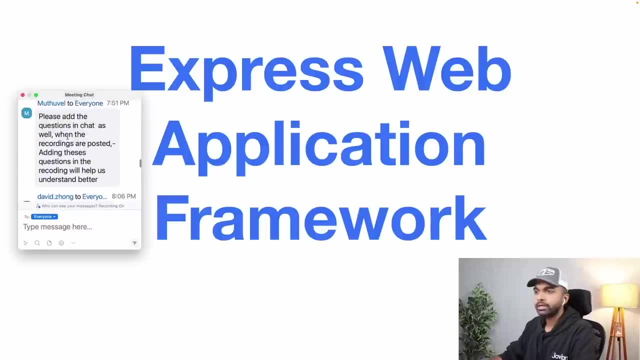 able to get some things out from the request, all the, all the form elements that have been sent, and then maybe do something with them, maybe send an email, send them to a database, et cetera. So there's a comment here. Well, a lot of things make sense now. Yep, Yep. 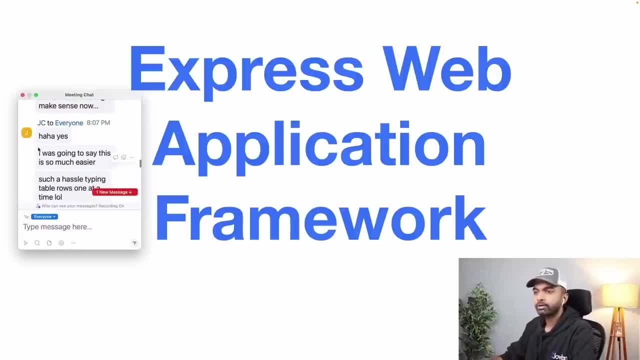 So this all fits together. We have to go about it, see, the whole thing to actually understand. And this was I was going to say. this is so much easier. It is such a hazard typing table rows one at a time, Exactly, So you almost never type out the data by yourself. 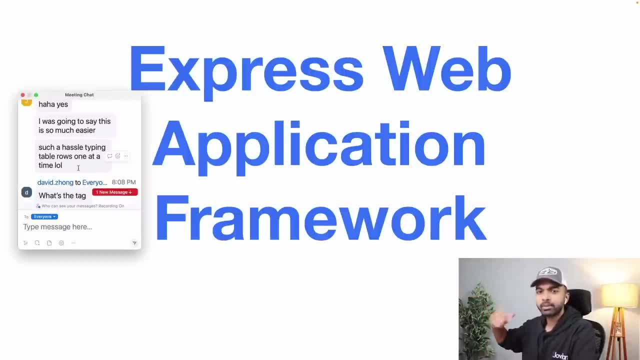 You almost always get it from a database and you just use some kind of a templating engine to just generate all that HTML for you. Okay, What is the small tag? Well, it simply makes the text a little smaller, That's all Okay. When do we learn to get data from the database? 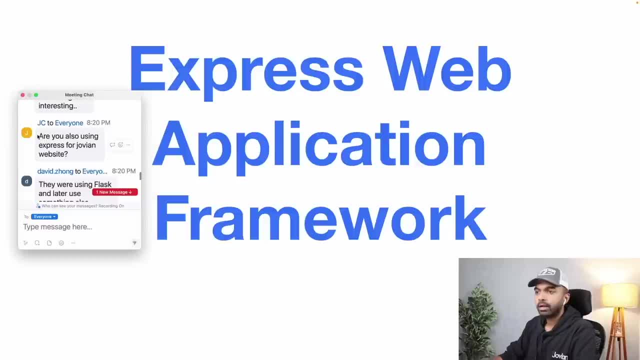 In a future course. are you also using express for the Jovian website? No, So we're actually using another framework called next JS, which is what is part of the next course, because we use a UI library called react and next year's plays better with react. A lot of people. 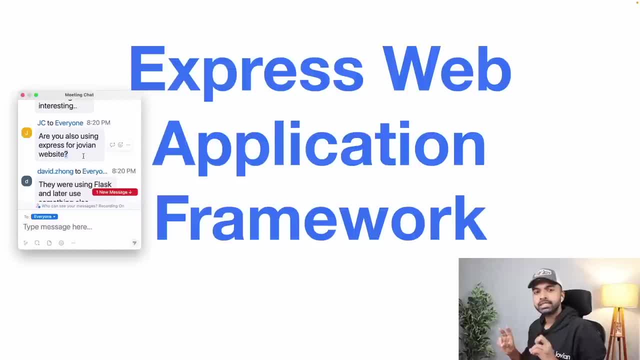 use express. It's part of this. You might've heard the mean stack, which is the MongoDB express angular JS and angular and node JS stack, I believe, or something like that. And similarly, there is a More than stack, which is the MongoDB express, react and node Yeah. So yeah, there are a. 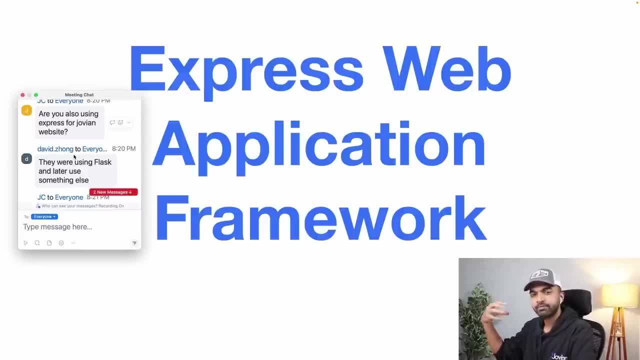 bunch of these stacks, but there's also some frameworks that are specific to specific UI libraries, for example, next year's, which is what we use, which is what we're going to cover. Okay, Then we were using flask and later using something else, So we're also. 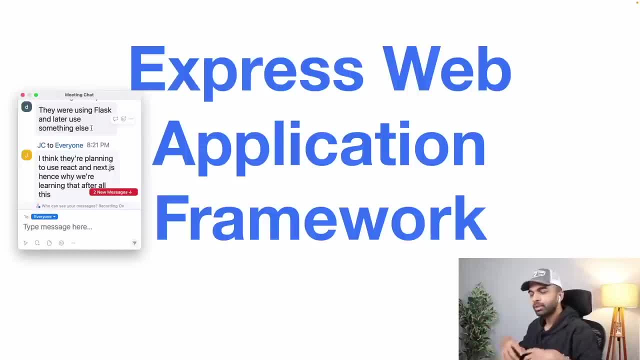 using flask for us. somehow, for some reason, we- because we've migrated to things over time. we started out with Python as our backend and X or Yeah. We started out with JavaScript as a front end, And that's why we still using both flask. 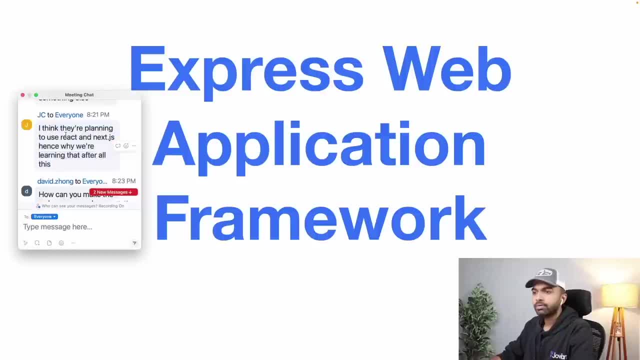 and next Yes, Okay, Yeah, So we are planning to use reactant. Yeah, We're already using reactant. They exist, We just haven't migrated to it fully. How can you make the web app Remember what you input? You cannot age. It's just that when you go back and forth in a browser, the browser 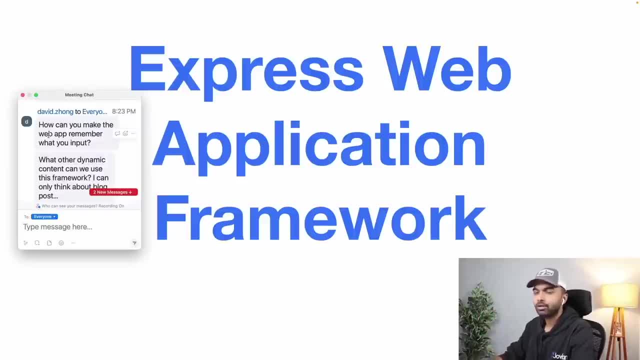 retains the history of the page. So that's all. I was just using that. normally, a web app will not remember what you inputted. What other dynamic content can we use this framework for? Well, you can create a blog post. All of Jovian could have been done, You can create. 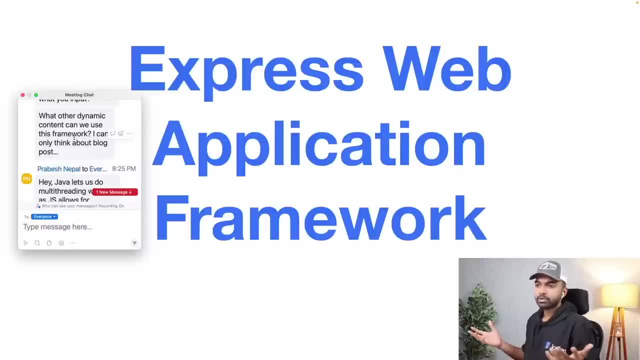 a blog post, All of Jovian could have been done. You can create a blog post. All of Jovian could have been built like this. There was no problem with it. Okay Is a Java lets us do multi-threading and JavaScript allows for asynchronous programming, but it is still. 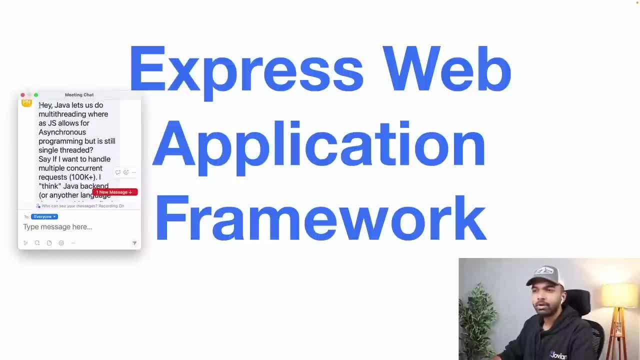 single threaded. Yeah, So this is some more advanced concepts. I will not really address this, but I'll answer your question. Say, if I want to handle multiple concurrent requests, I think a Java backend would do better than a JavaScript. Well, not necessarily because 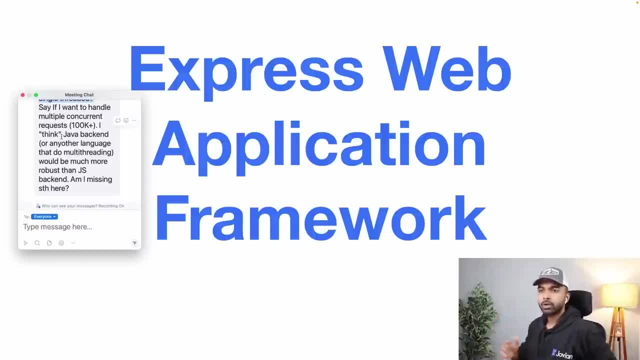 what you could do is you could run multiple JavaScript processes. So what do you do is JavaScript itself is single threaded, But what you can do is you can run five JavaScript processes and all of them can asynchronously handle a lot of load for you, Or you could. 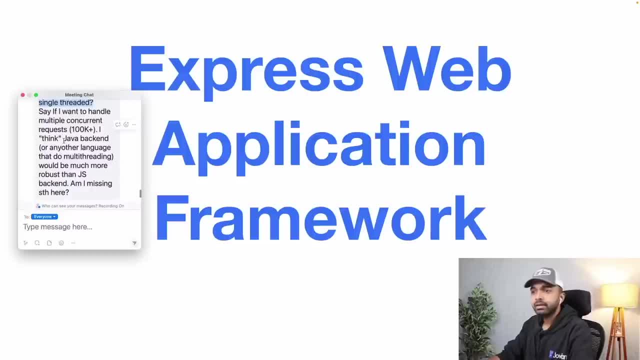 just use a bunch of servers. That said, a Java backend would be better if you have to do a lot of processing on the server. Typically if you simply have to call a database and then return the result, maybe just formatted in a certain way. fill out a template: Nodejs. 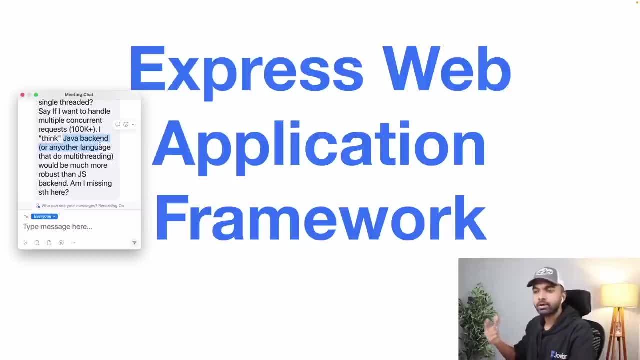 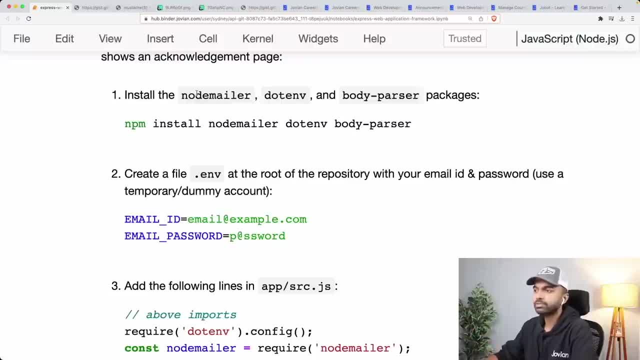 of things, So this is a Java backend. You can do a lot of things, So this is a Java backend. the person who, who applied, just so that they know as well. but in any case, now for that, we are going to use the node mailer package number one. second, we are going to use a package called dot env. 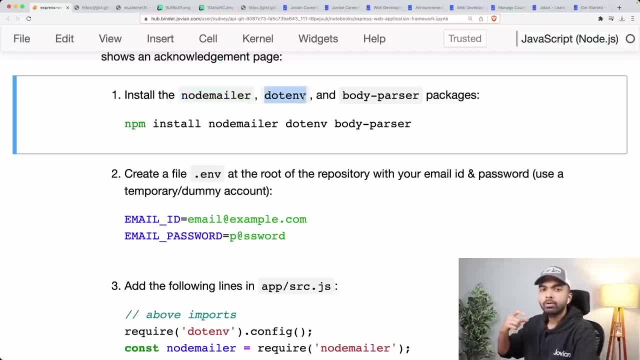 now the dot env package is useful when you do not want to put sensitive information, like your email password, in the code. remember, we are going to put up all the code for this particular email, for this particular project on github, in public, or sometimes even in private, and we may not want. 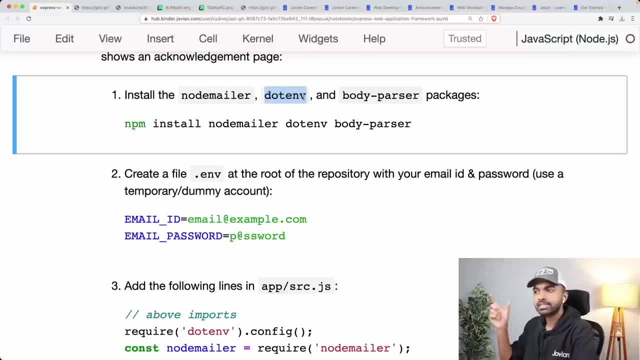 to put our password there, because then our password will just be present there on github for everybody else to see. so that's where there's a way to securely read some of these things using environment variables for which we use the dot n package. and finally, the request body that is being 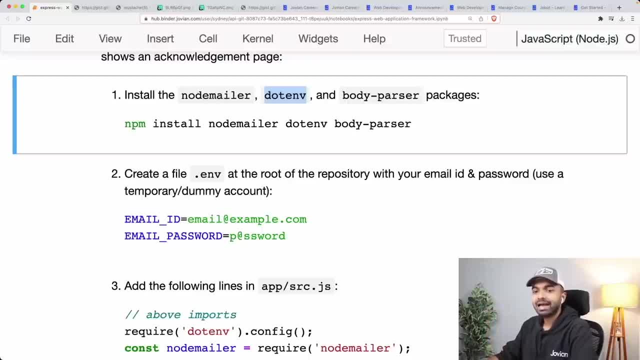 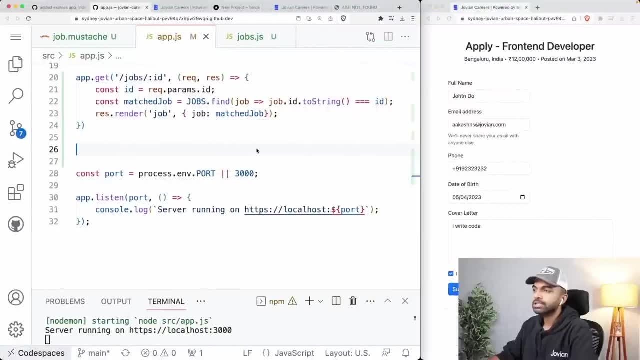 sent, when we are posting the form data that that body is going to need to be passed in some way, and for that we need to use this body parser package. okay, and you'll see all of them in action shortly. so let's come back in here. let me shut down the server for a second. 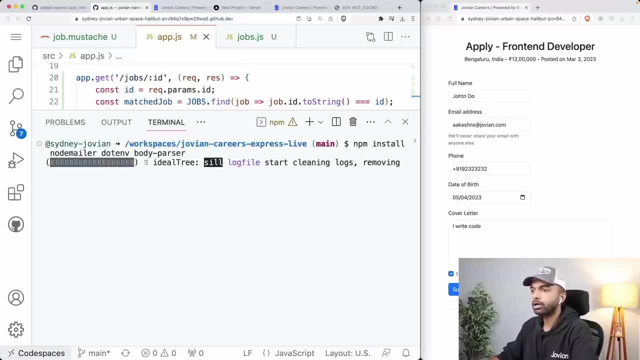 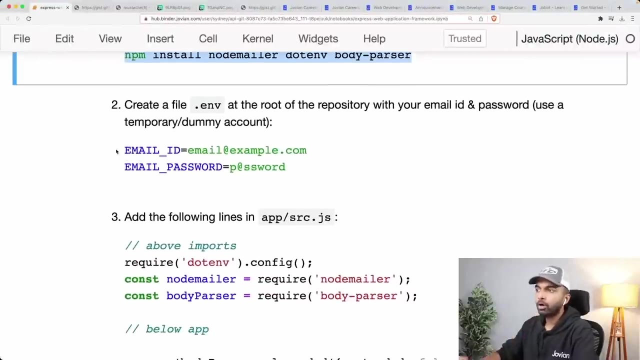 and let me now just install these packages: node, maler, dot env and body parser. okay, all the packages are installed. now i can restart the server, npm, run dev, and let's close this for now. next, let us create a file called dot env at the root of the repository. 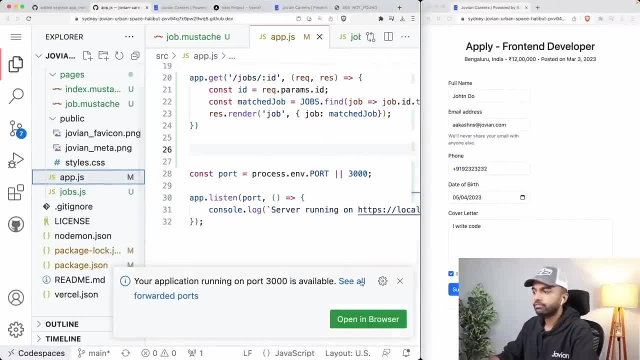 so i'm just going to open up the pdf ahead of time and save it, and now we will be able to see. So I'm going to create a file over here called dot ENV, into which I'm going to put in my email and password credentials. 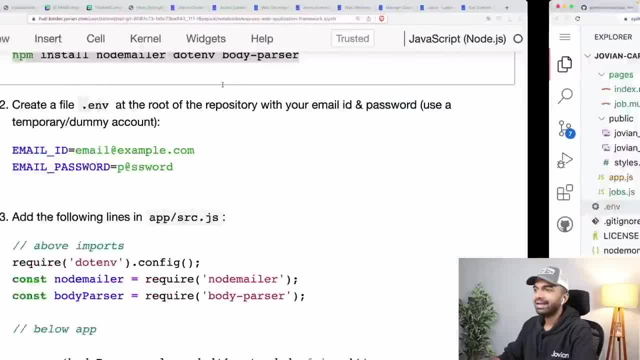 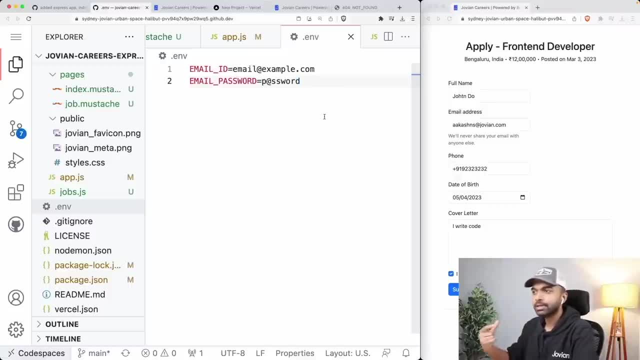 So let's put in a folder dot ENV in the root of the repository And into this I'm going to put in these two things. Of course, what I'm going to put in here is the actual email and the actual password that I want to send the data to. 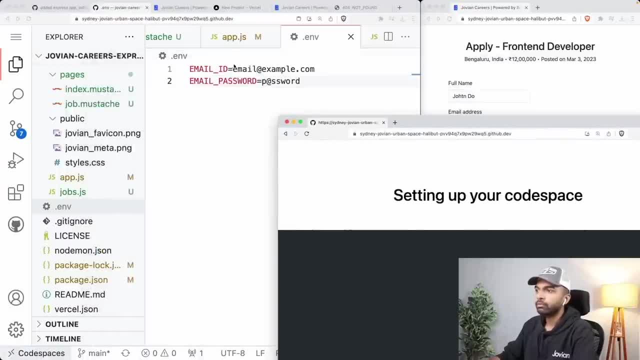 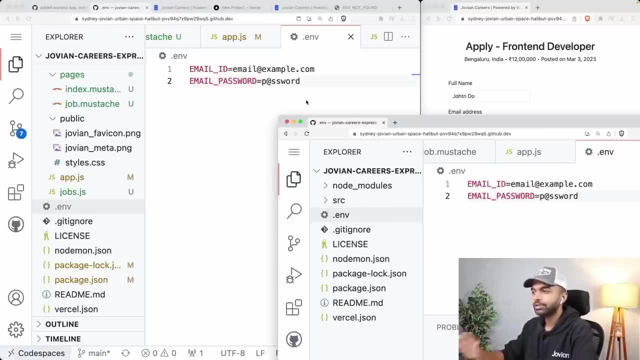 Um, obviously I don't want to show you that information, So what you will have to do is you will have to replace this with your email and your password, And I would suggest not using your primary email. uh, just to be careful. 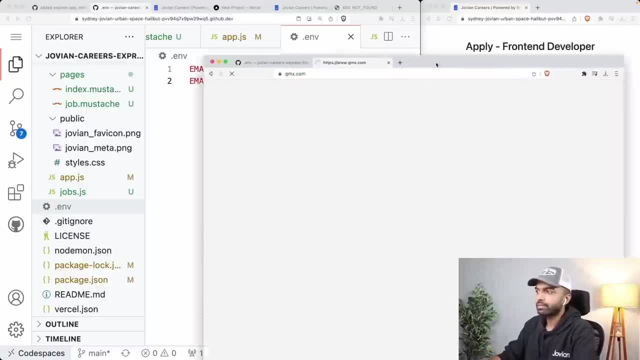 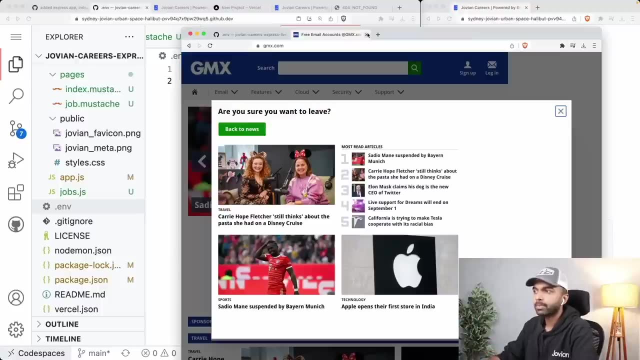 What you can do is you can go to gmxcom. This is a website where you can create a free email, and on gmxcom you can just create an- uh, a throwaway email and just use that and its password. Okay, 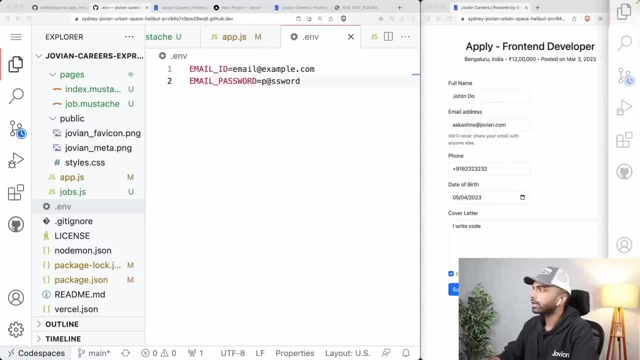 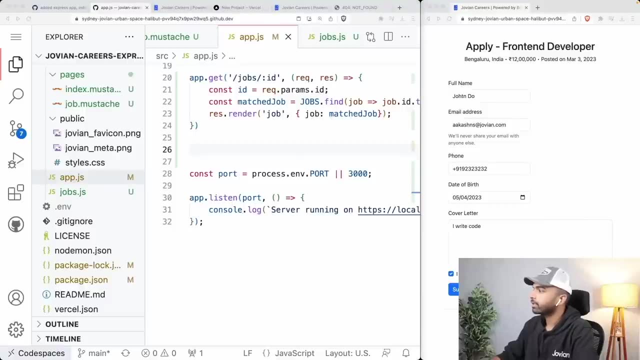 And that's what I'll be using as well. So I'm just going to go in into another desktop over here and I'm going to close it over. close it here, But I'm going to put in my email ID, which I have created for this tutorial. 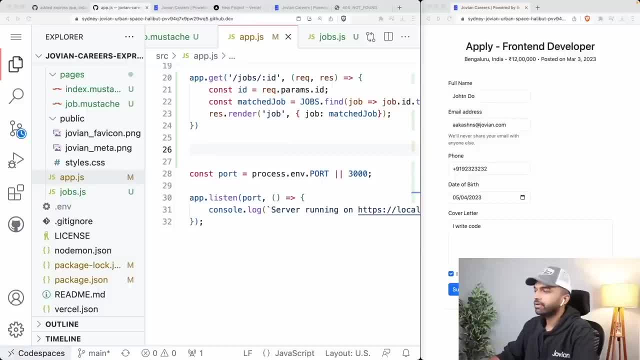 And password. Okay, And I've done that, So I'm not going to show you my ENV file again. If I open it, you will be able to see my email and password. So I won't show it, but it's there. 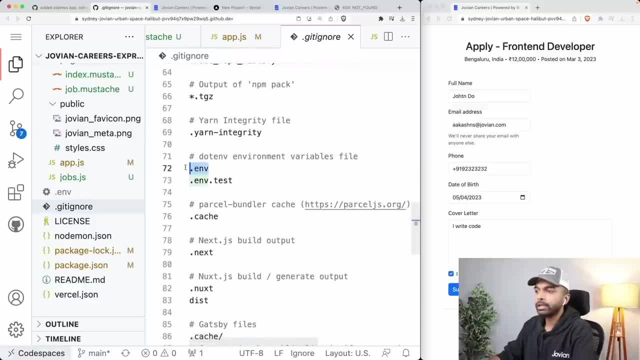 Now, the other thing I want to mention is the ENV file is already ignored in the dot get ignore file. So which means when I do a git commit and send it to GitHub, then this data is not going to be sent. It is going to remain securely on my code spaces machine, which is just private. 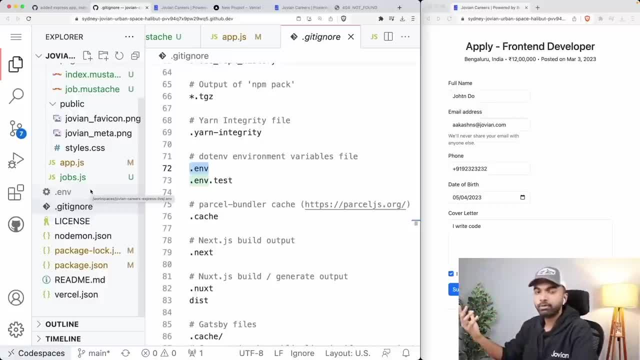 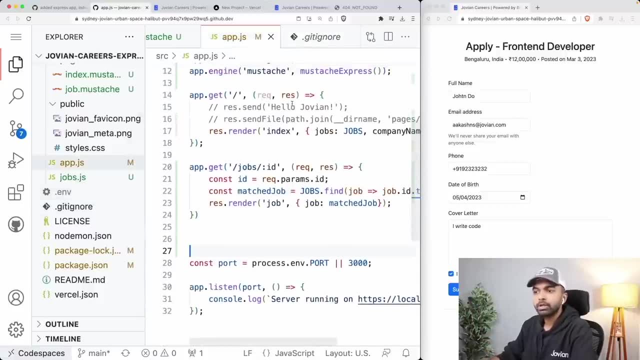 for me and it's not going to be sent to the GitHub repository, which is public for everyone to see, Or if it was private and my coworkers would be able to see it, which is again undesirable. Okay, But now that we have put the information in this dot ENV file, we need a way to 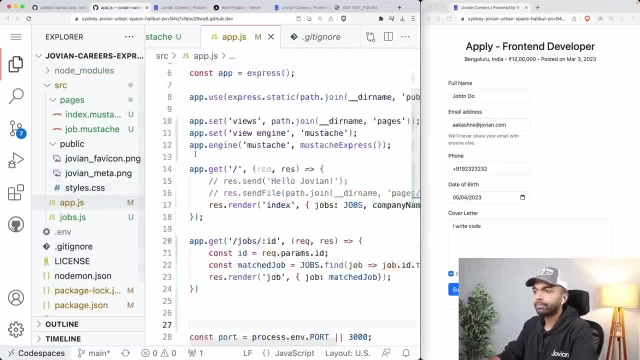 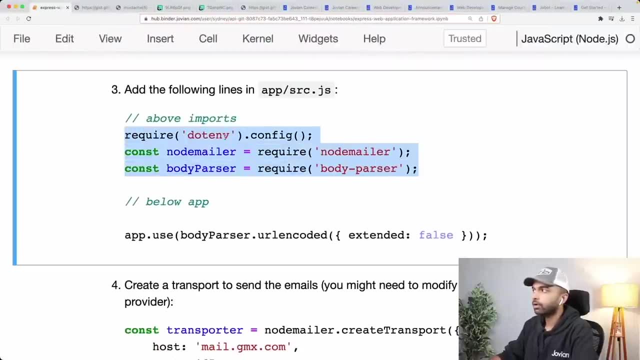 actually load this information into our app. How do we load this information into our app? We do it by saying this: require dot ENV- dot config. So the first line, require dot ENV- dot config, is going to read the dot ENV files that are present in our project folders. 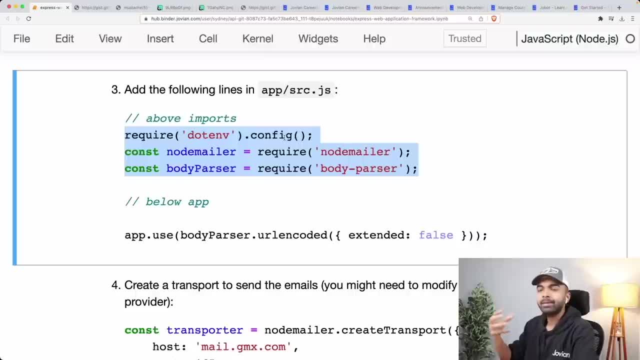 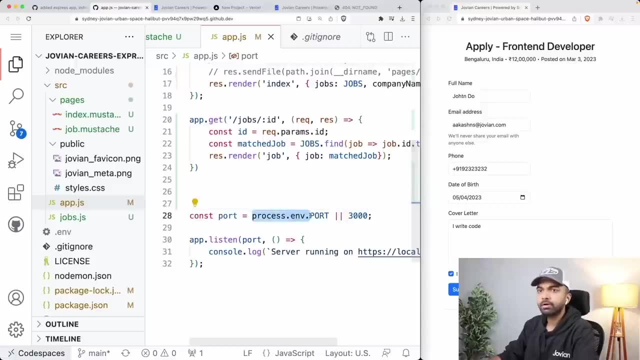 And it is going to then read each of those and then automatically add them to the process dot ENV variable. Okay, So remember we had this process dot ENV variable. So now, instead of apart from dot port, it can also get a bunch of other things that we have defined. 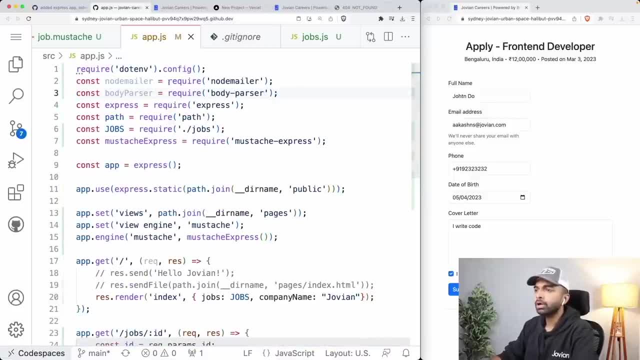 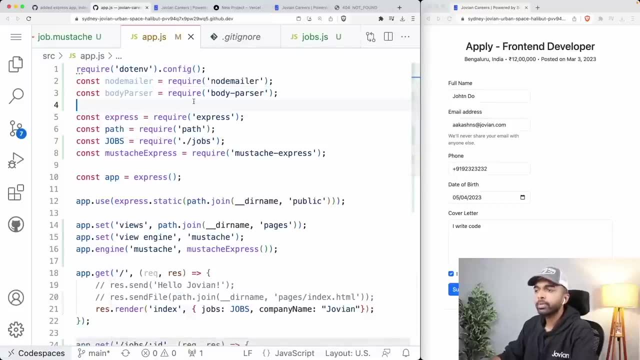 So let me just put this right here at the top dot ENV. And now here we have the. we've also included the node mailer package, and we've also included the body parser package. Okay, All right. Next step is to also. 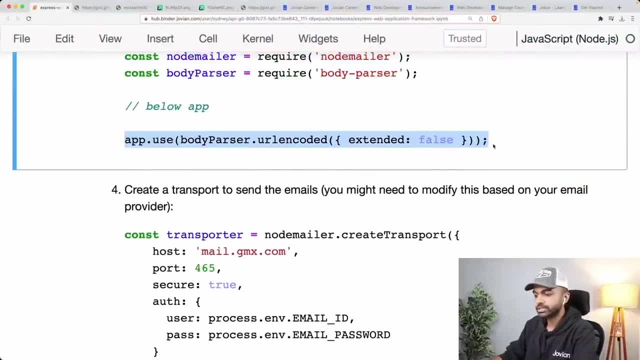 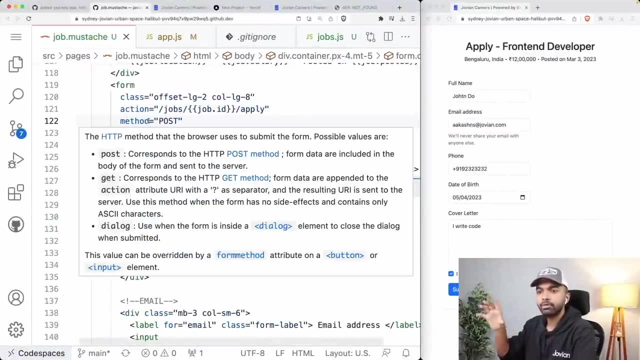 Also configure our application to use the body parser. So remember, when we send the data from this form, we are posting it, which means we are not sending the data in the URL We, which means we are actually I'm sending it in the body of the request and that body of the request. 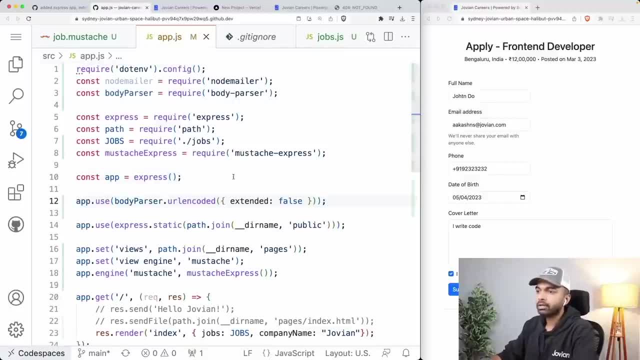 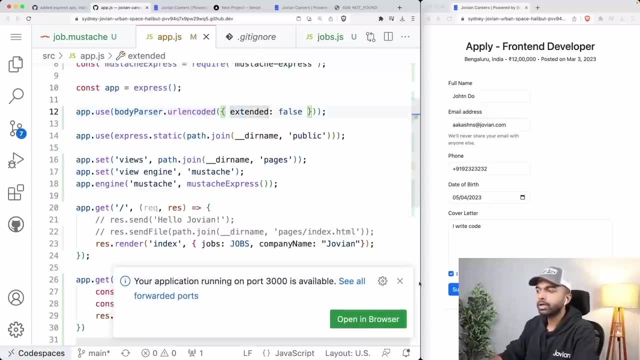 needs to be parsed in a special way. The right below app dot express, light below my app creation logic. I'm simply going to say: app dot use body parser. dot URL: encoded, extended, false. Now, don't worry about All of this right now. if you just search online how to add body parser to express. 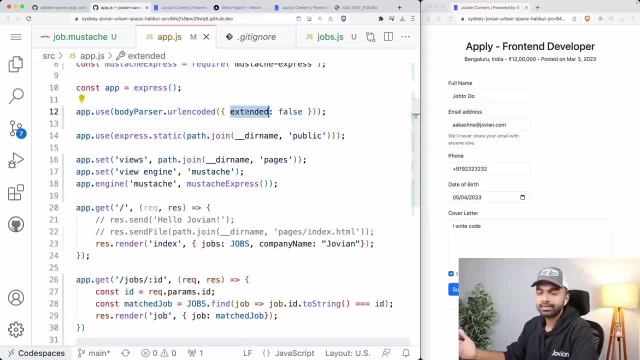 you will get the line of code that you need to add and you can look up what exactly extended does. Okay, But the basic ideas and, by this, one general tip I want to give you, that is, From this point on, you will see a lot of code which we are using. uh, which? 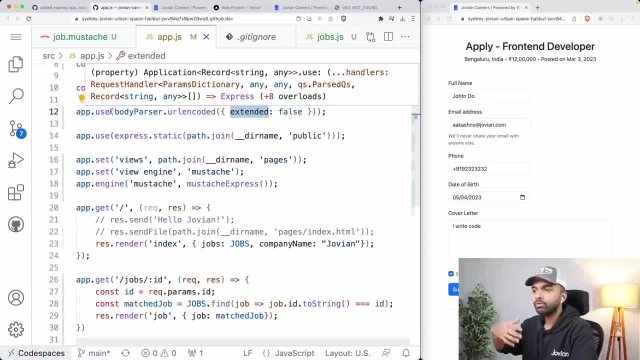 we will not exactly describe perfectly, And the idea is that you have to kind of look it up online- maybe use chat, GPT, job board, Google- and understand what it means, because there are so many libraries, so many frameworks, so many. 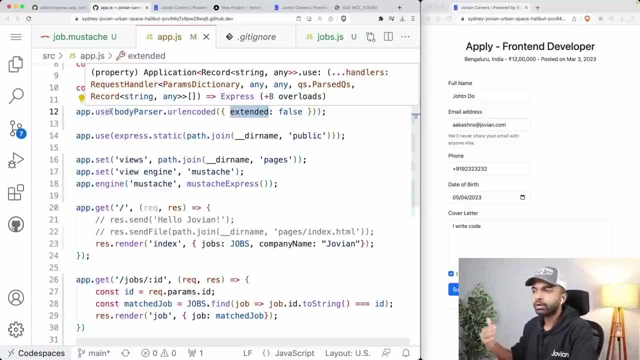 Uh, options in each of them that it doesn't really make sense to cover all of them. It's something that you should just look up, uh, and try to figure out as you need it. Okay, So now we add body parser. 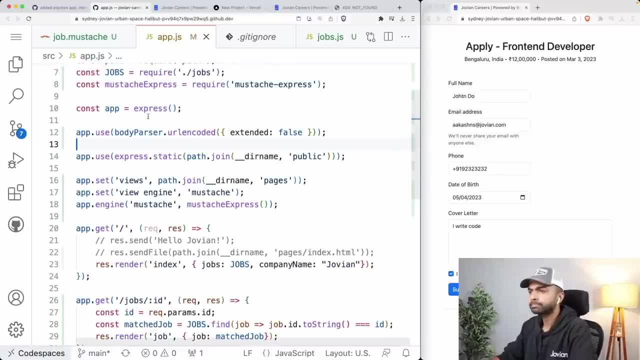 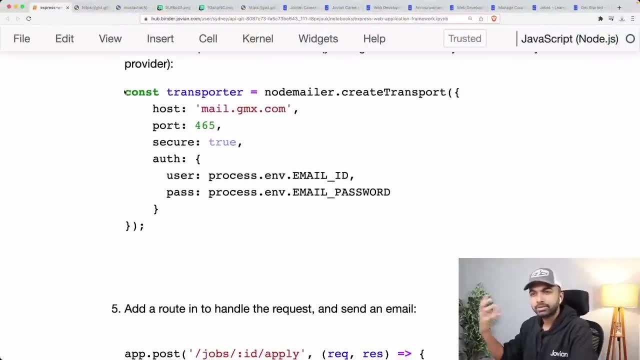 We've added this middleware essentially to our application to, or, which is going to pass the request body. And now, uh, one other thing we need before we actually start processing the request: we are going to create a transporter. We are going to create a transporter which is going to have the configuration required. 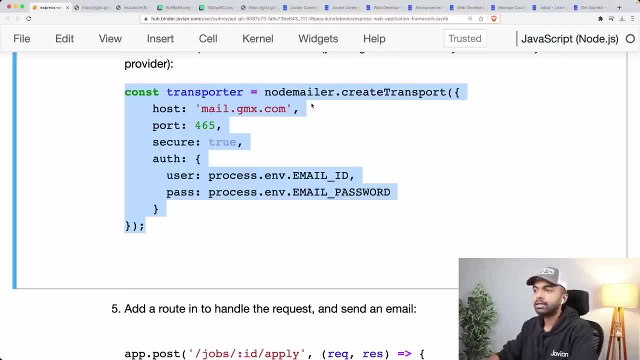 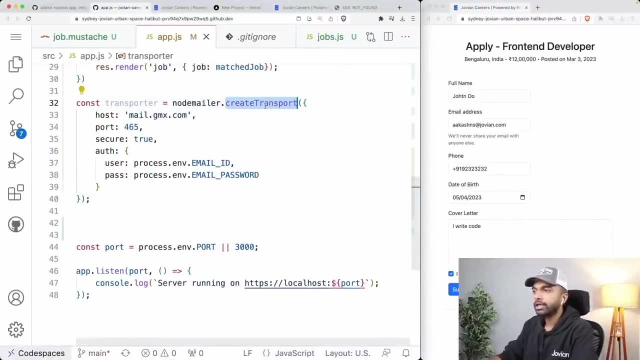 to Connect with the mail server and send the email. Okay, So I'm let me create this transporter over here. So I'm going to say no more, no mailer dot create transport. And this transport, uh, is basically it needs, it needs a host. 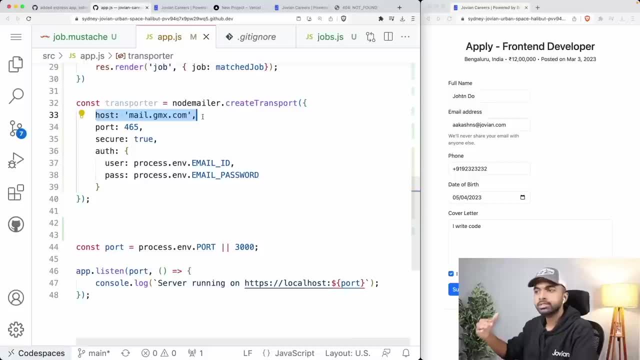 The host is mailed, or gmxcom. So, depending on which email provider you're using, you'll have to look up their SMTP host. So just search for SMTP host or your email provider And you also need to look up their SMTP Port. all right. 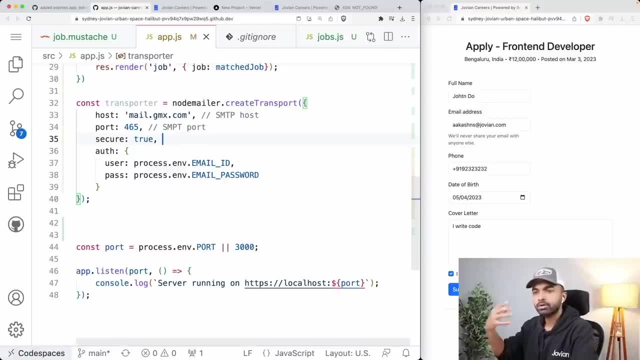 And then, finally, your secure true is almost always set. secure True means you're using HTTPS, the secure version of the transport, And finally, you need to provide authentication and in the authentication you need to provide the username and the password as a user and pass keys. 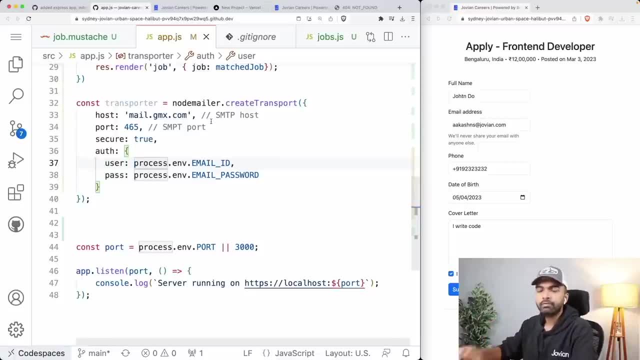 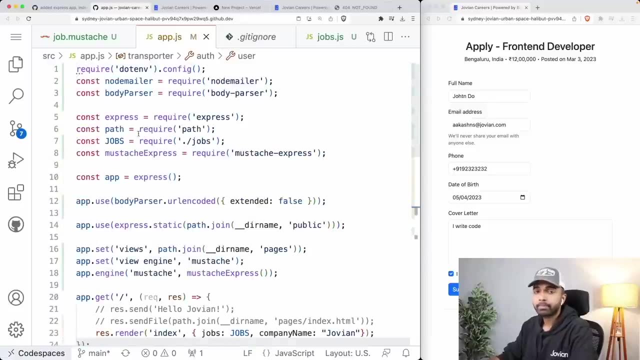 Now, of course I'm not going to type in my username and password here, rather, since I've already put something into the dot ENV file and I've read that using the dot ENV require dot ENV um line of code over here. 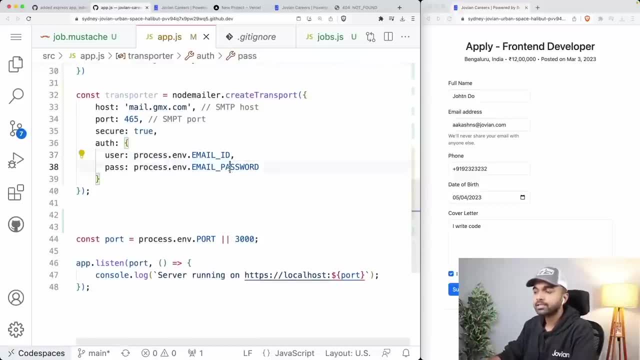 So this is automatically going to get populated, Populated with my email ID, And this is automatically going to get populated with my email password. So now we have this transporter and now we can simply say transporter, dot send, and that's going to send whatever email we want to send. 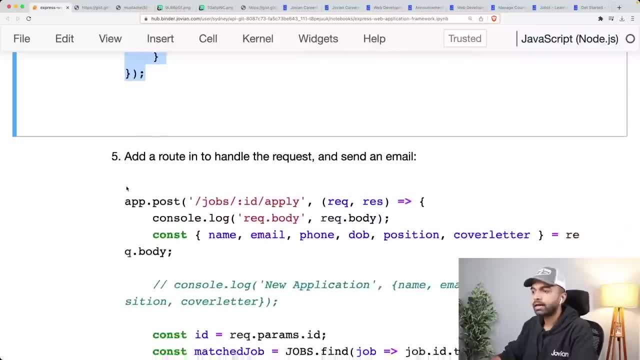 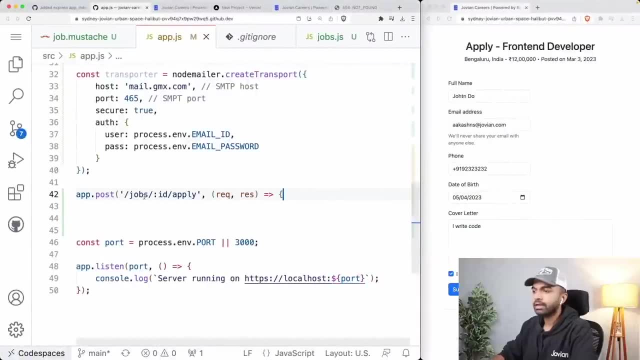 Okay, So with that we are finally ready to actually pass all the content. So let's just go about this line by line. So let me come in here first and let me just for now Simply say: Console dot log. request got body. req dot body. 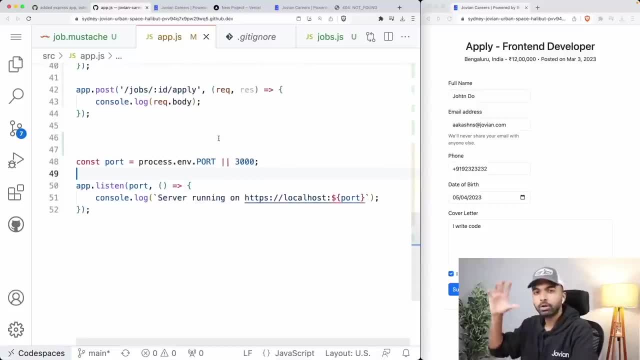 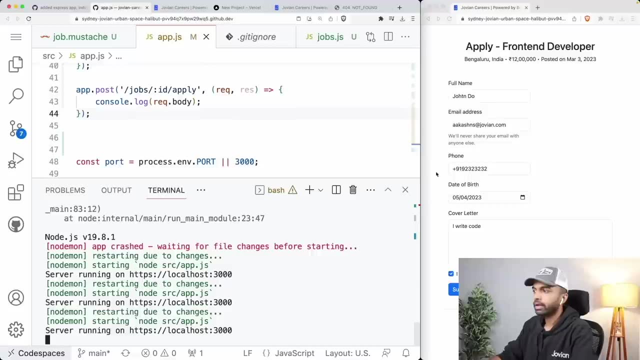 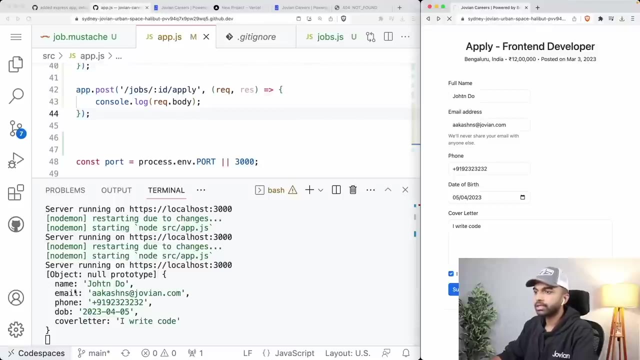 All right, Let's just do that much. very straightforward, We're just going to log the body over here, So let me just open up the terminal- This is my terminal over here- and let's just click submit application. And you can see that when I click submit application it simply said um name: John John Doe email. 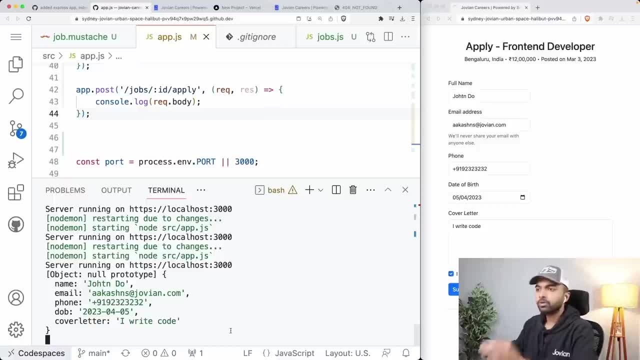 whatever a car should joincom phone number, DOB, cover letter, et cetera. So we simply logged the body over here and nothing happened here because we have not sent anything from the server. Let's just go back, Yeah. 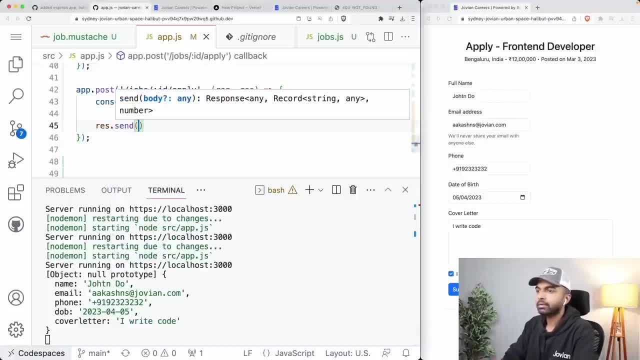 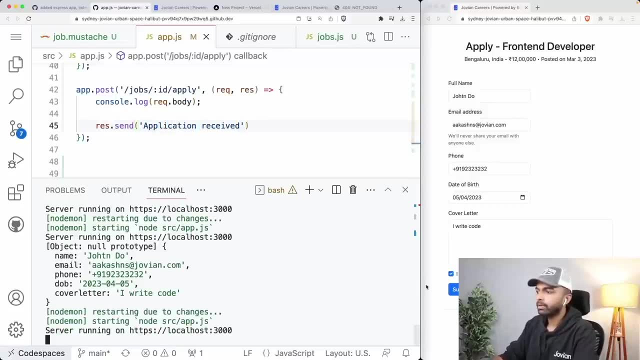 What we can also do here is: we can. we can do right now: rest or send application received. If we had done that, then when I click submit application, it's going to log the request body over here. You can see it logged the request body over here for us. 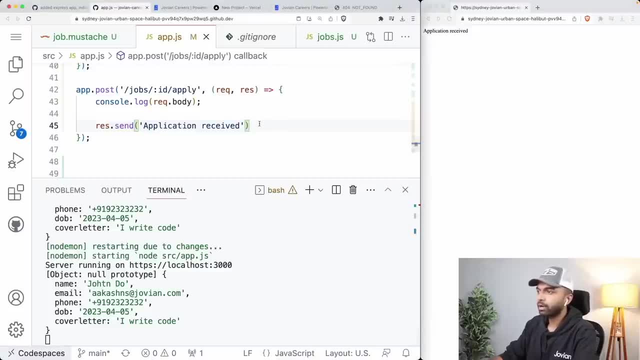 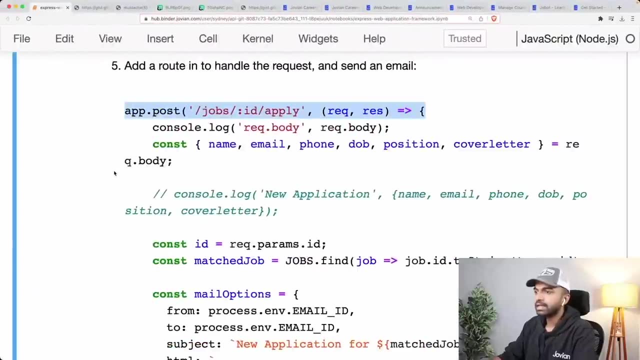 But along with that, it also Printed application received. right, But that's not what we want to do. We want to actually do something with the application. now that we have the request body, Okay, So what next? Well, next up, then, let us get. so. the request body has this name, email, phone, date of birth and cover letter. 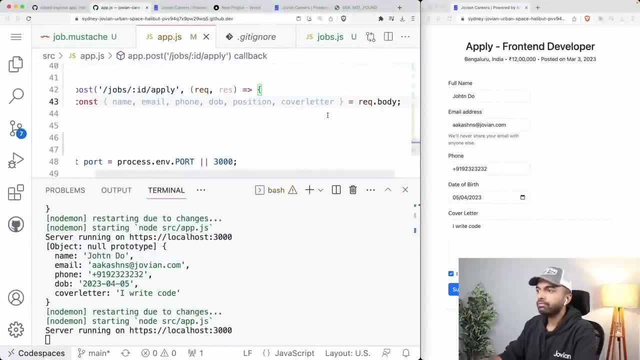 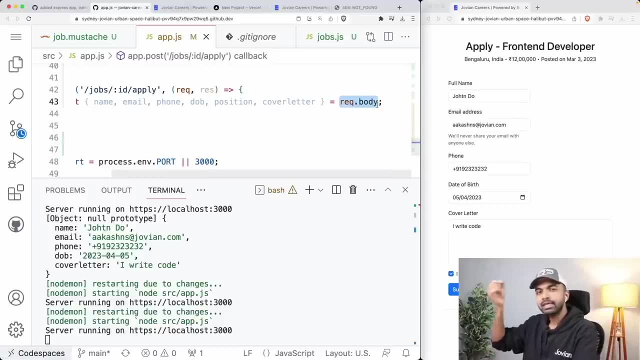 Let's get all of that information out from the request body And for that we're going to use this special syntax called destructuring, Whenever you have a particular object and you want to get the keys out of that object, and you know the names of the keys. 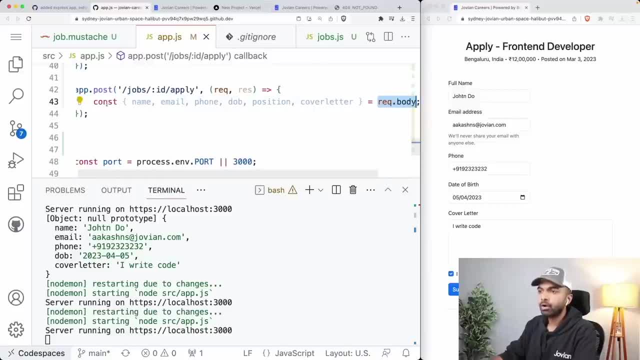 you can put all those keys into specific variables like this, So you can say const and then you can open brackets and then type the names of all the keys that are present in the object. Or you can pick just some of the keys that are present in the object. 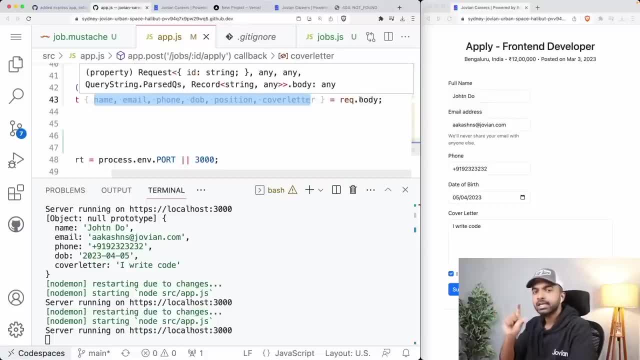 And you can say equal to requestbody. So it's kind of the opposite. Instead of saying requestbody, equal to name, email, et cetera, Now you're saying that from requestbody, extract the name and put it into a variable called name. extract the email, put it in a variable email and just do that. 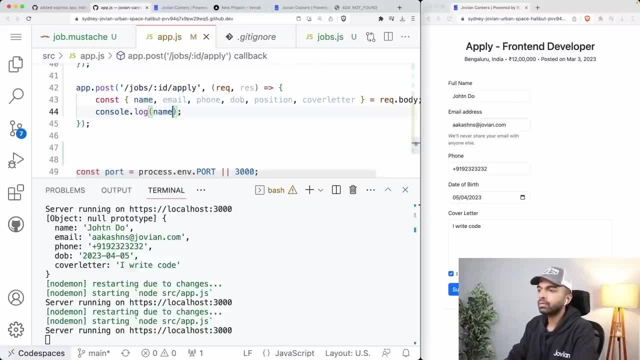 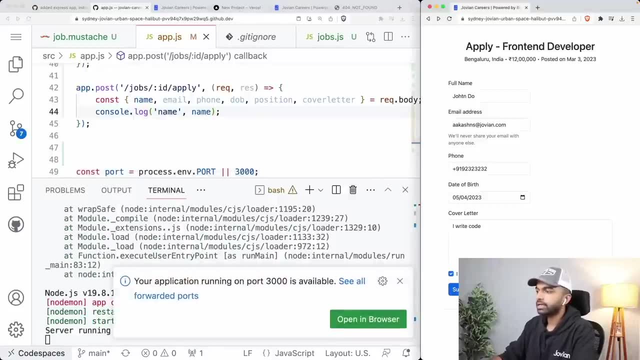 And now you can see if we do consolelog name. Now this will just have the name picked out from the request body. All right, And I can see submit application here. Yeah, If I say submit application, you can see. it prints the name John Ditto. 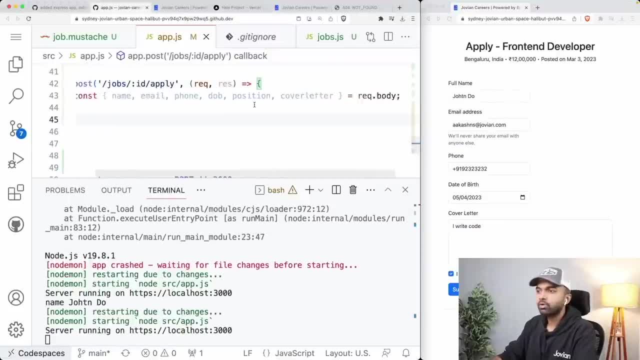 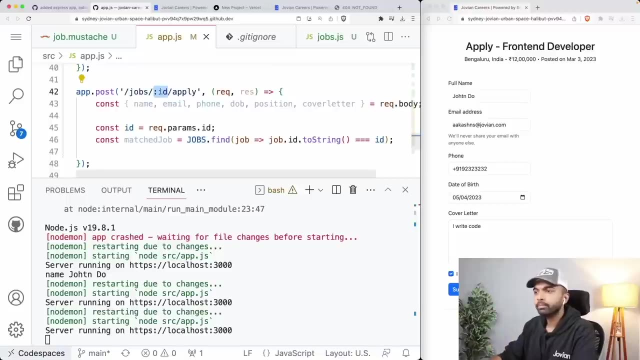 Okay, So we now have all this information from the request body into a bunch of variables- Nice. Next, let us now get the job that we are currently working with. So remember we are posting. When we are Posting, We are also specifying the ID of the job in the URL as a route parameter. 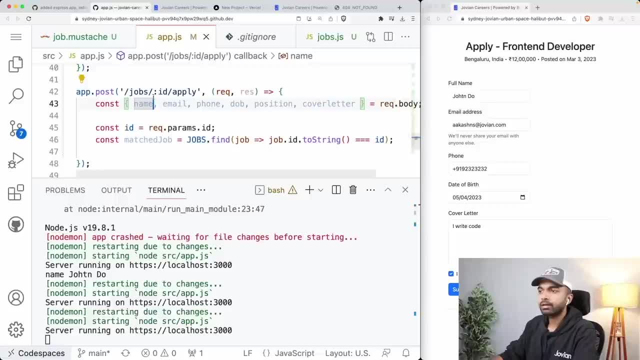 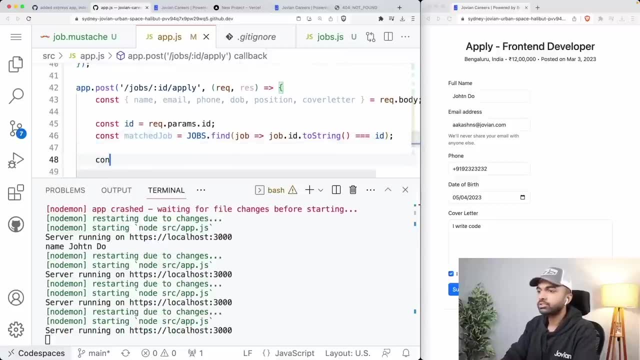 So let's get the requestparamsid. that is going to get this, that is going to get this URL parameter ID and let's get the matching job. So let's also print in the matching job. So let's log consolelog: matched job. matched job. 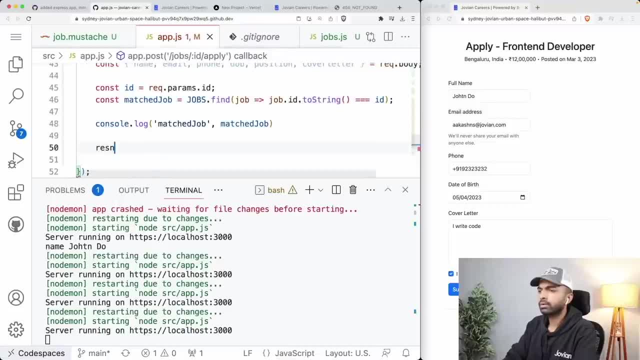 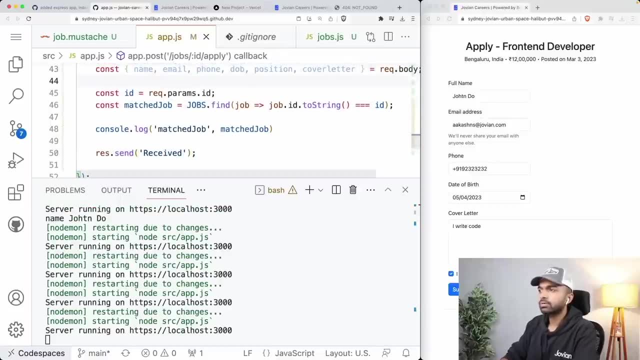 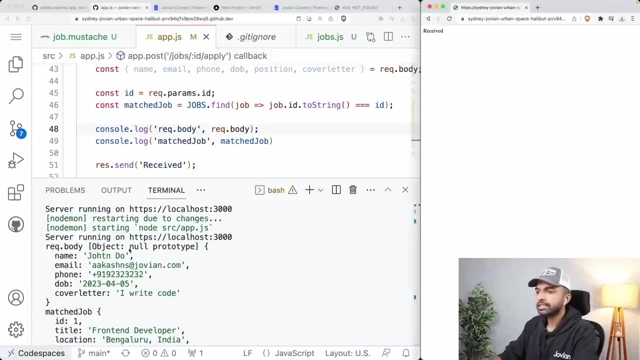 Okay, And let's also for now just do restsend, So that is a match job. but then let's also maybe log the request body, just just for complete clarity. Okay, And let's click submit application once again. So now you can see that this was what was sent or submitted by the user. 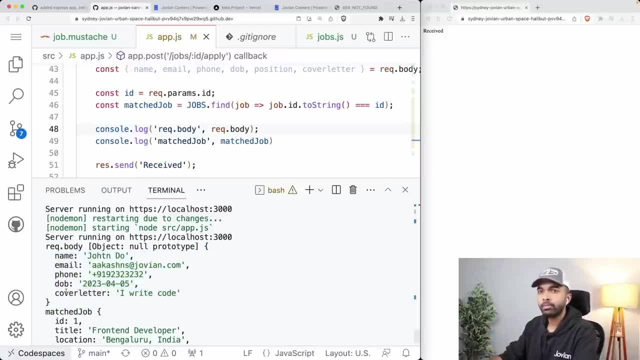 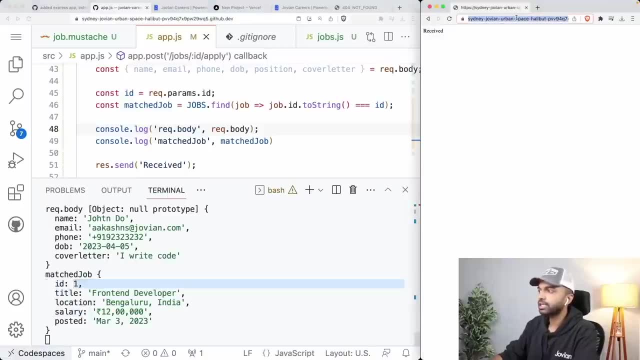 So this is obtained from the form that the user submitted name, email, phone number, date of birth, cover letter and this was received. This was a match Job, So that means in the URL we had slash one. If I check the URL over here you can see that we've done slash one, slash apply, right. 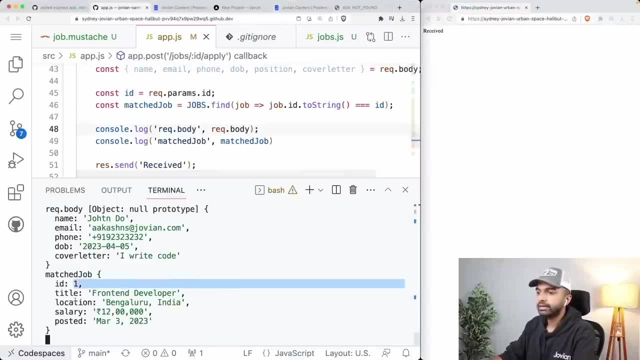 So slash, one, slash apply and that is getting picked up as the ID here. So and that has been matched or searched within the jobs list, which currently comes from a file but could have come from a database, And from there we get the title of the job. essentially, 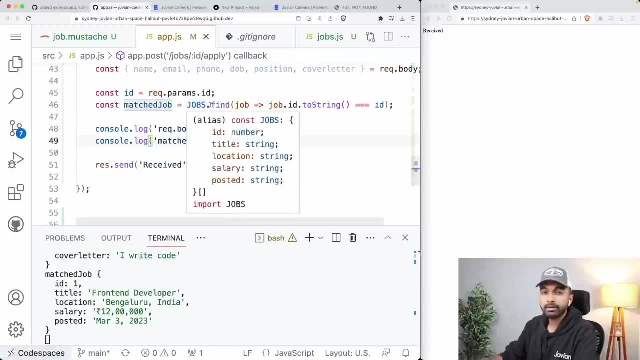 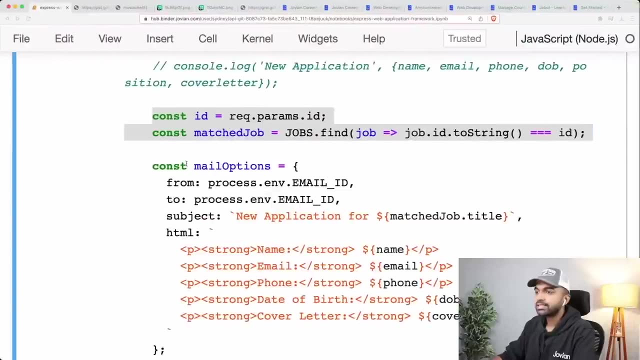 So now we have all the information. We have the information about the job that that is being applied to, we have the information about the application, We have the information about the application itself, the applicant itself. So the next step is to actually construct an email. 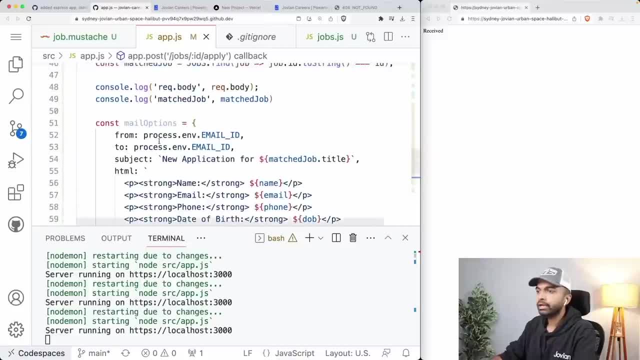 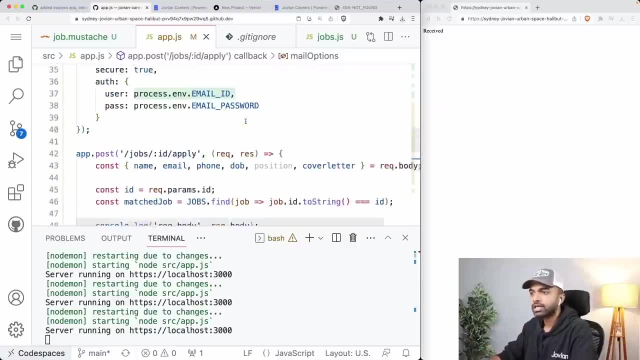 So for constructing an email, we create this mail options object. All right, So all we're doing here is into it. We are putting a from email Now. the from email ideally is the same email, that whose password you have put in into the transporter. 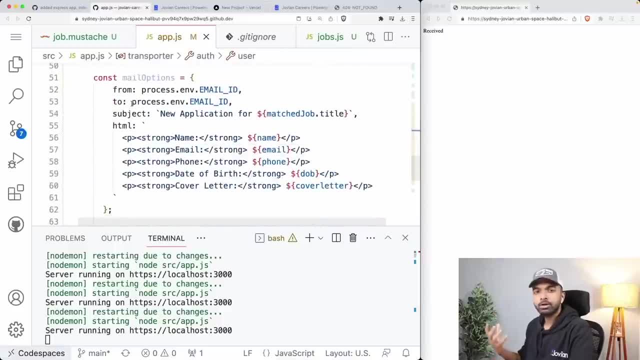 So, yeah, you put in a username and password, So the from email should be the same. The two email could be whatever you want. Let's say you've set up this GMX email. You can put your credentials or put your password of the primary email. 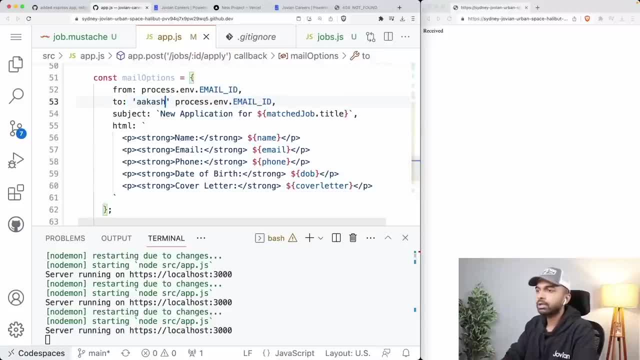 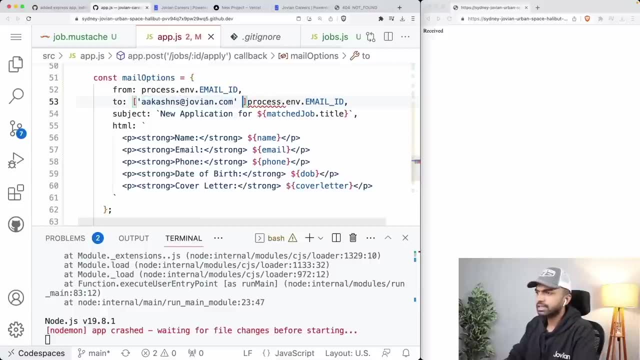 The two email could be. I could put into the two email. I could just put in Akashns at jobiancom, something like that, or I could also put in: I believe I could put in a list as list here as well. 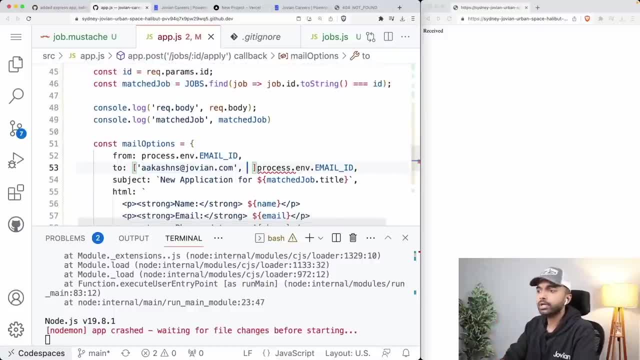 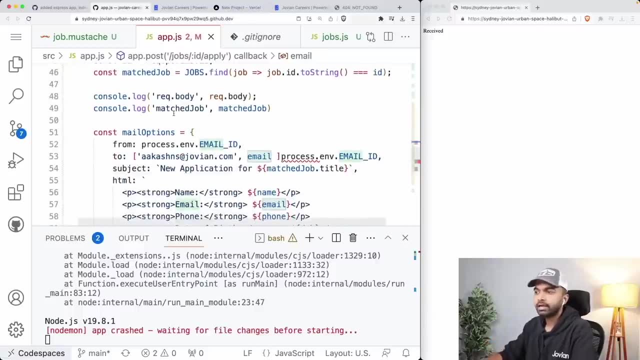 So let's say I also, apart from sending it to myself, I also wanted to send it to the person who has actually emailed me. So their email is present now in the email variable, I can pick it up from the application and I can email them that the application sent and such and such. but for now, just to keep things simple, 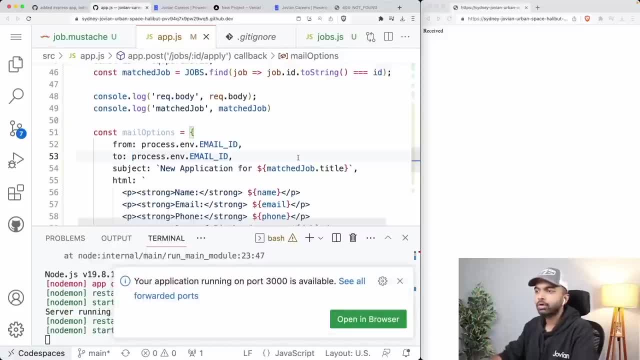 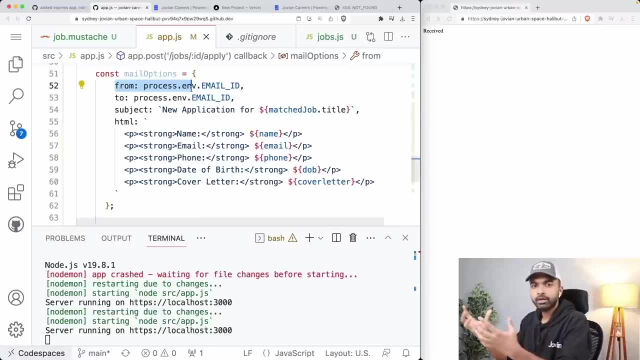 I'm going to send it to the same throwaway email that I've created. All right, I don't want to worry about that, but I could send it to whatever email I wanted. So keep that in mind. from is ideally the same email that you've configured in the transport to can be whatever you want. 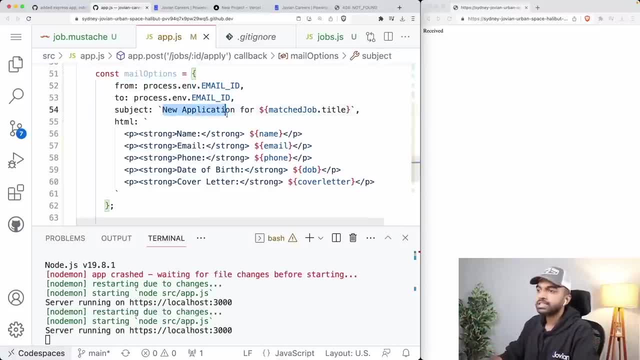 You can put in multiple emails here as well. All right, Then we have a subject we can set, and I'm just saying new application for match jobtitle, so that when I get the email, I want to know which job the person is applied for. 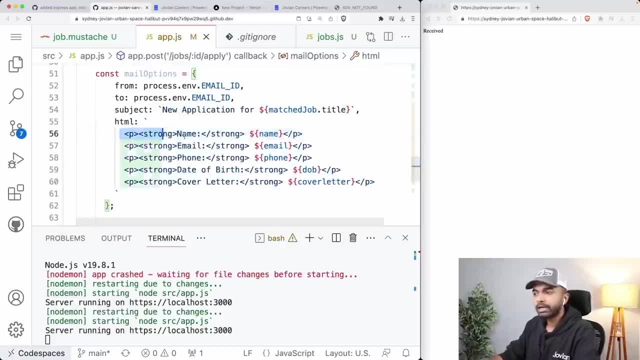 And then you can create some HTML. So what you can do is you can create an HTML. So what you can do is you can create an HTML. So what you can do is you can create an HTML string and inside that HTML string we have inserted a bunch of these things. 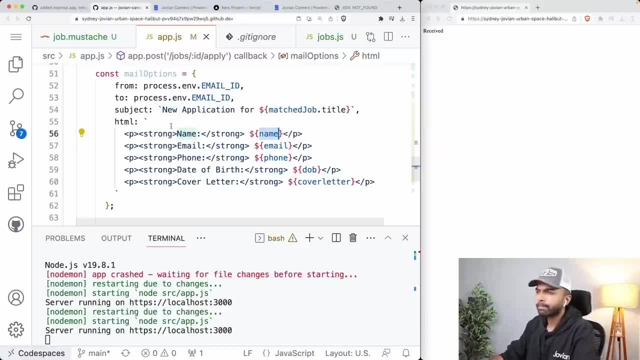 So this is what is called a JavaScript string formatting, essentially a template, literal, where you started with a back coat and then you insert into it using a dollar. You insert name, email, et cetera. Okay, You can learn about this. 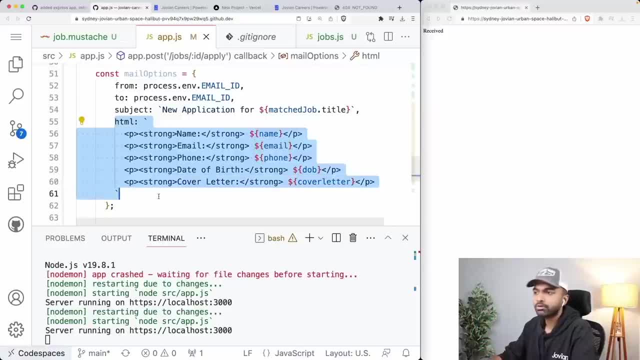 What are you going to do is? you can also just paste this code on chat, GPT or job board and ask it to explain the code, But essentially what we're doing is we are creating a simple HTML email with name, email, phone number, date of birth and a. 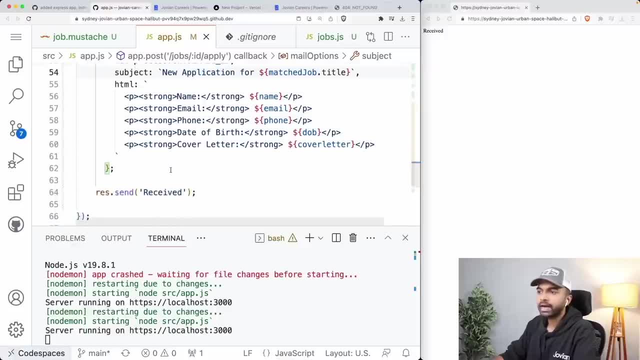 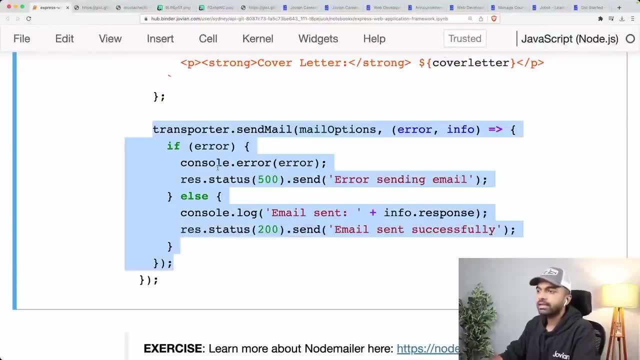 Cover letter, information or a name, email, phone number, date of birth, cover letter, all of that And that is our mail options. So with that, our mail options object is ready And finally, we can now just simply send that using transporter. 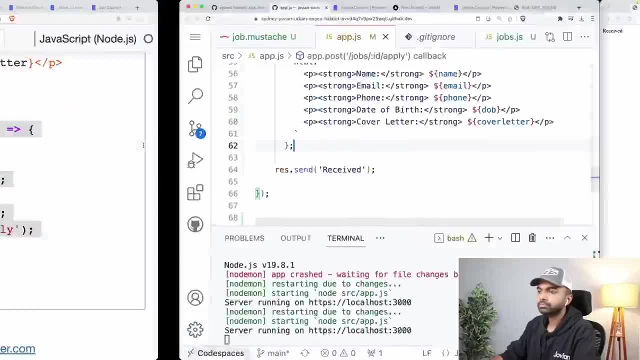 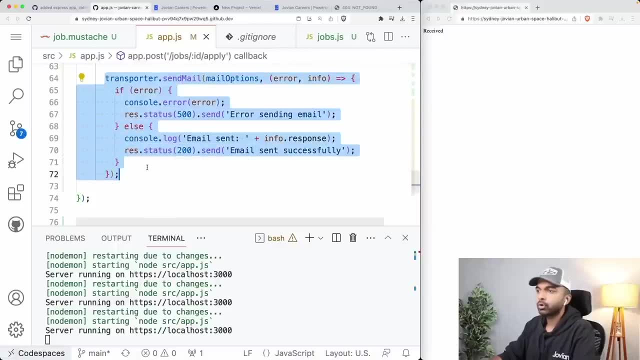 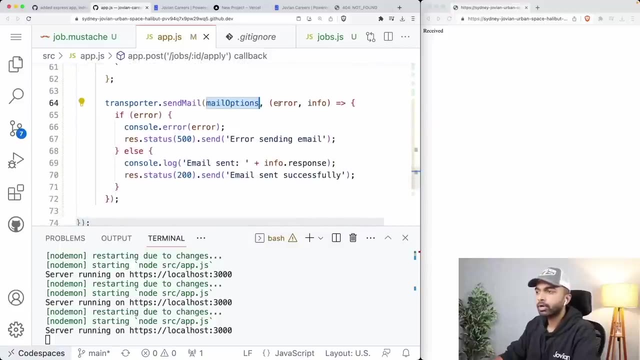 Now we can say transportersend mail. Yeah, Now let me get rid of this restsend and let me paste this in here. So now we can simply say transportersend mail and I give it the mail options, which contains the from to subject and HTML body. 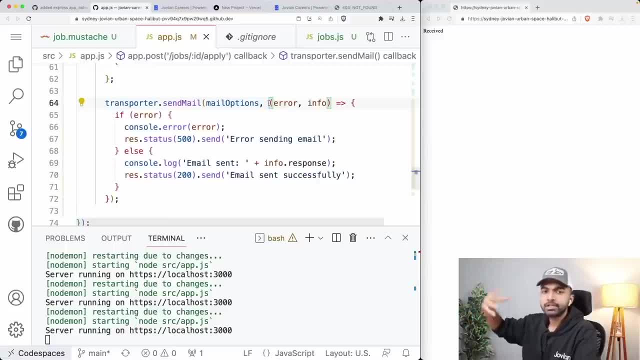 And then I can give it a handler. So when it tries to send the mail and let's say it succeeds or fails after the mail sending is done, it is going to get called. It is going to call this handler function that is provided here with whatever error or info was received. 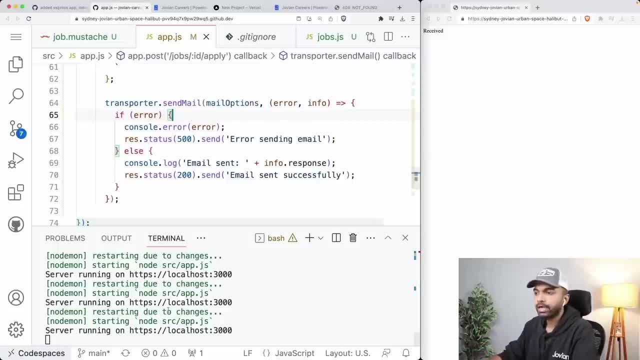 So if there was an error, then we want to simply log that error, We want to print that error here in the server And we want to say: error sending email. If there was no error, then we want to simply say: email sent successfully. 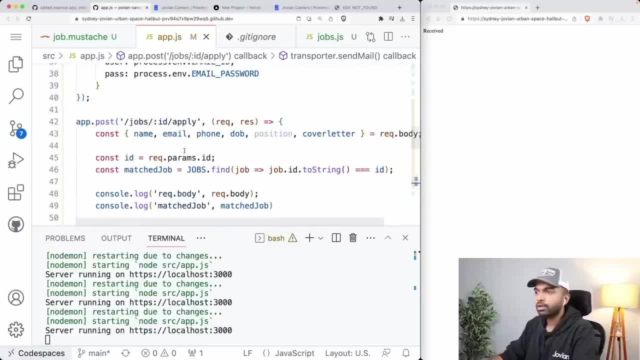 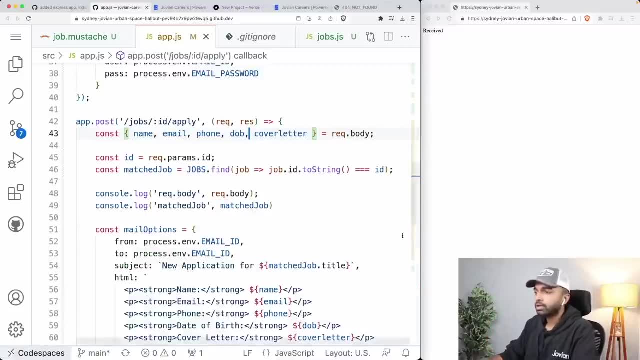 Okay, So let's just save that. Um, so now we have all the information. I think this position is Not required because we are not actually asking for position in the form. Okay, So I'm going to just close this terminal tab here. 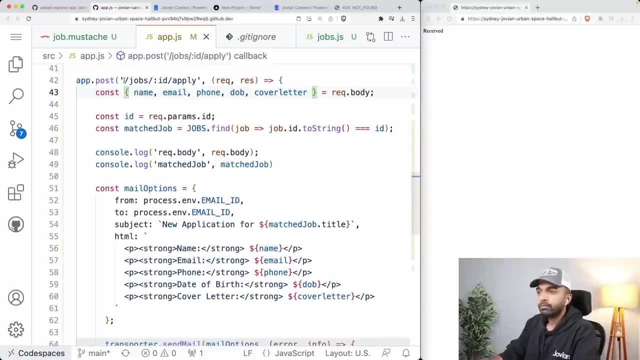 Let's take a quick look at this again before we actually run it, for when we post some data to slash jobs, colon ID: slash apply- Then this handler gets called from the request body. We are going to get the name, email, phone number, date of birth and cover letter from the request params dot ID, which is the URL parameter. 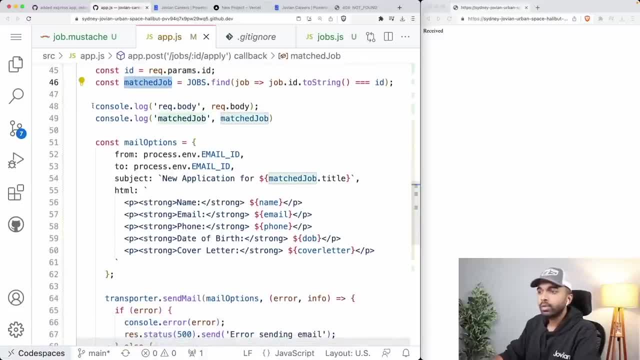 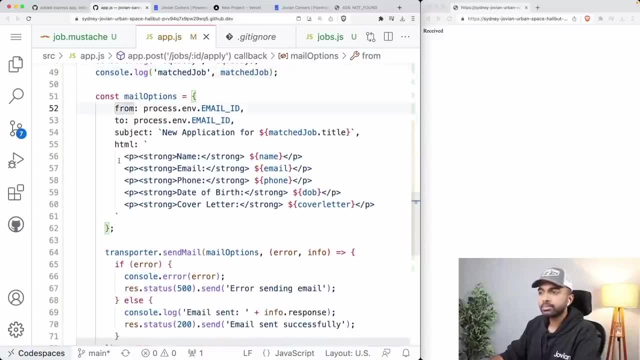 We are going to get the ID and we're going to find the matching job. We are then logging both of them to the terminal And then we are creating a meal options which contains a from two subject and a body. And then we are saying transporter dot. send mail with the mail options. 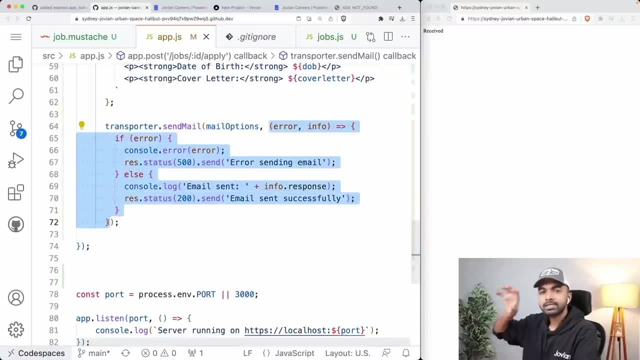 And if we receive an error, so we need to give it a handler. So what happens is it tries to send the mail in the background And once the mail sending is done, it calls this handler function. So you always have this like callback function that you keep passing to almost everything that you do in JavaScript, right? 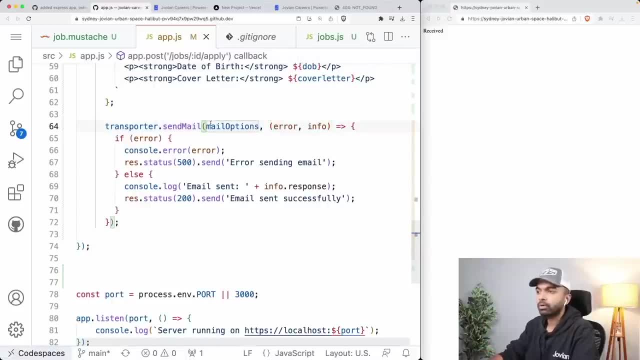 This is. this is what is meant by asynchronous programming. That you're not. you're not blocking the main thread. You can serve other requests from other clients till the meal is being sent in the background, And then, whenever the mail sending is done, it is going to invoke this function. 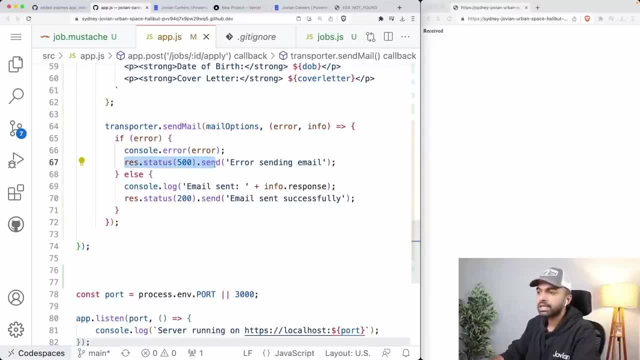 Now, if there is an error after sending the email, then we are going to say rest or status 500, error sending email. So what we are saying by status is HTTP status codes indicate whether the request was served successfully or not. So I would encourage you to just search for HTTP status codes. 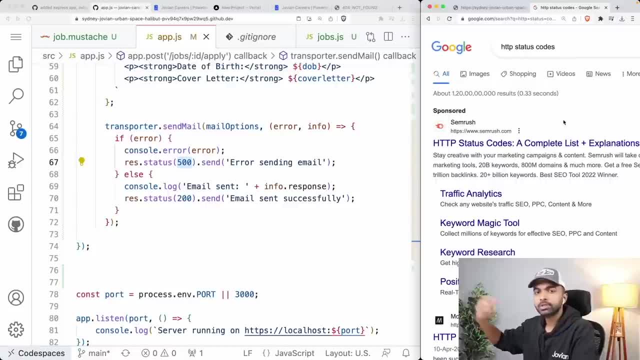 No, you must have heard of 404,, which Is that the page or the URL was not found. 200 simply means that the URL was found, 500 means that the server encountered at another, 400 means bad, request means you made some mistake by sending the request, and so on. 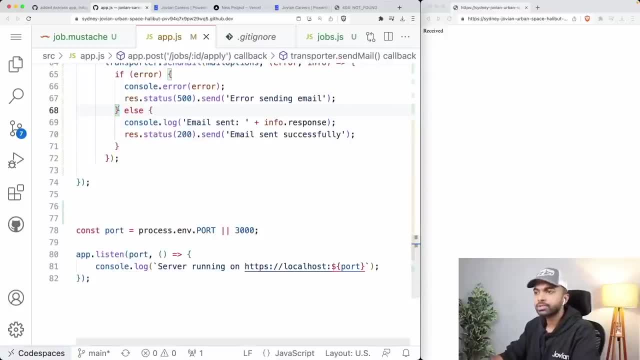 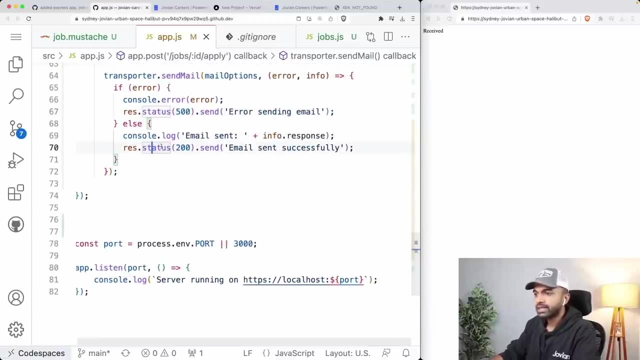 Right. So there are all these HTTP codes that the server uses to inform the client what went wrong, if anything, Okay, And it also sends a message error sending email. Otherwise, it says rest or status: 200: email sent successfully. Okay. So let's now go back here. 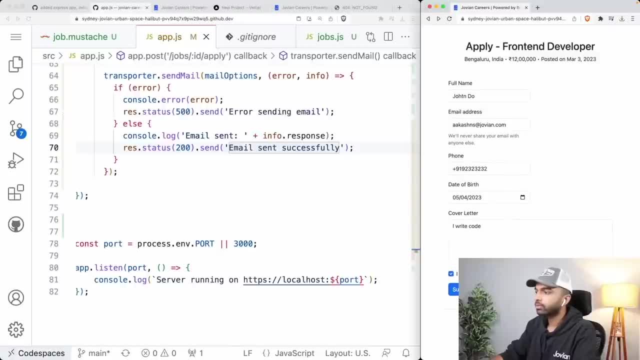 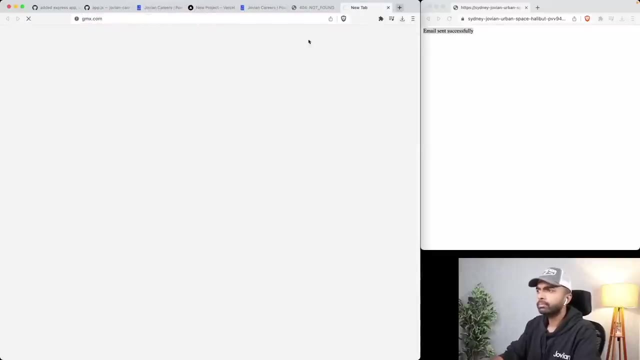 And Let us submit this once again. I'm going to click submit application. This is the moment of truth, And when we click that, it says email sent successfully. So I'm just going to go into my GMX account. So gmxcom. 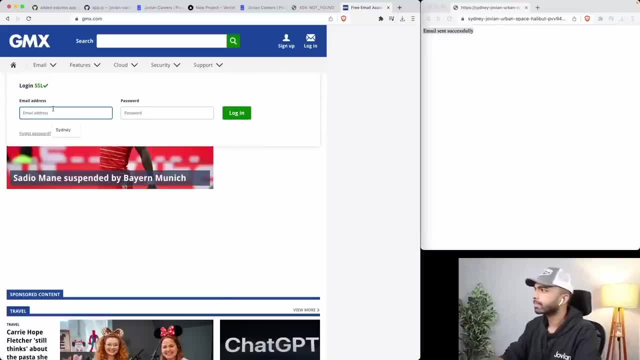 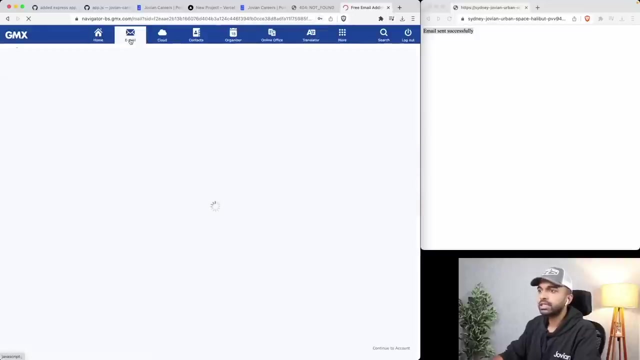 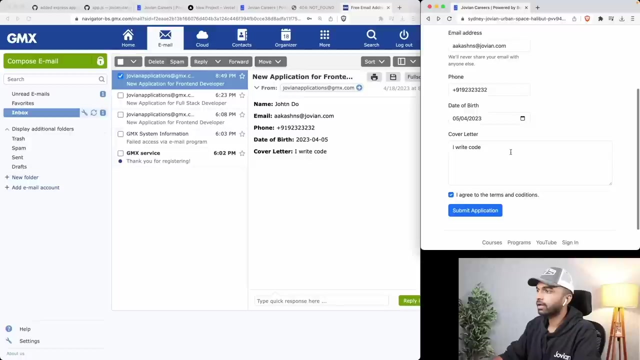 And let me just log in over here. Let's see. Let me grab my email And password and let me log in. and once I am logged in, hopefully I should be able to see that new email. but it says: your new application for front end developer, John D John Doe Akashns at joviancom, phone number is such and such, date of birth is such and such. I write code. well, that seems to be exactly what I had filled out here. 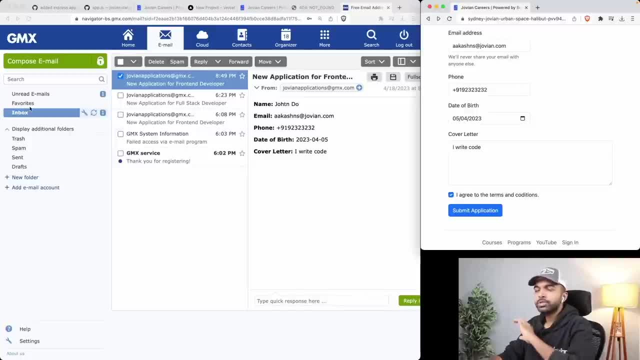 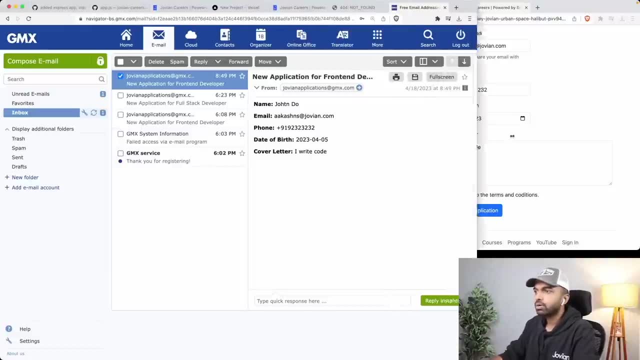 Great, Now, one thing I want to mention. I want to mention, though, almost every email provider has turned off SMTP by default, because it is somewhat insecure, and that includes GMX too. So what you, what you will need to do first is, if you're using GMX, you will need to go into home. 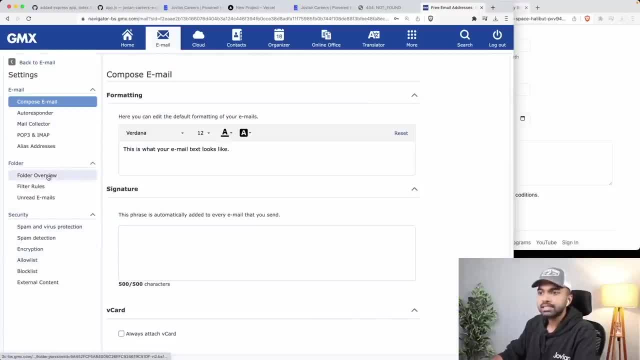 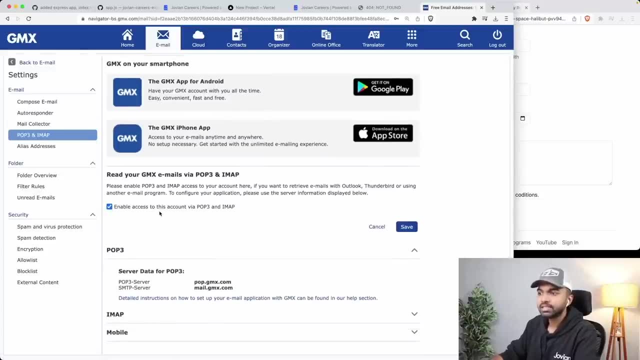 You will need to go into email settings and under email settings, you will need to go into pop three and IMAP and under pop three and IMAP, you will need to enable the setting: enable access to this account via pop three and IMAP. 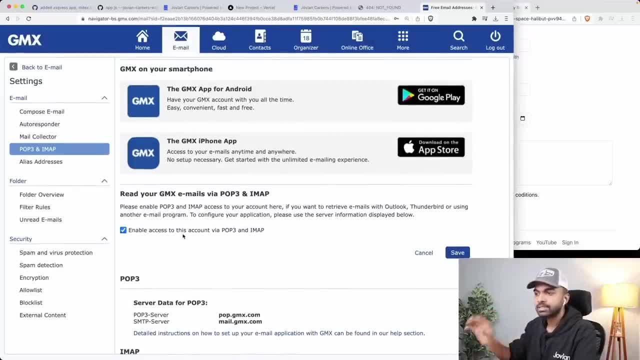 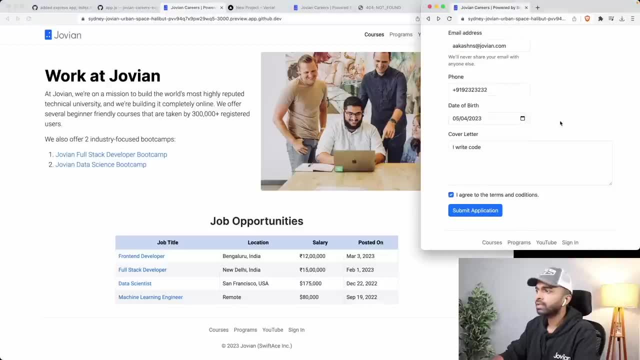 Okay, So that is just how. So that is just how you enable this SMTP business on um GMX. Let's see if it's not enabled. So let me just show, show you what happens if I don't enable it. 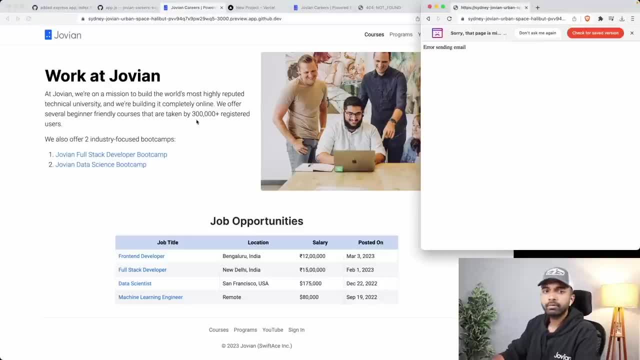 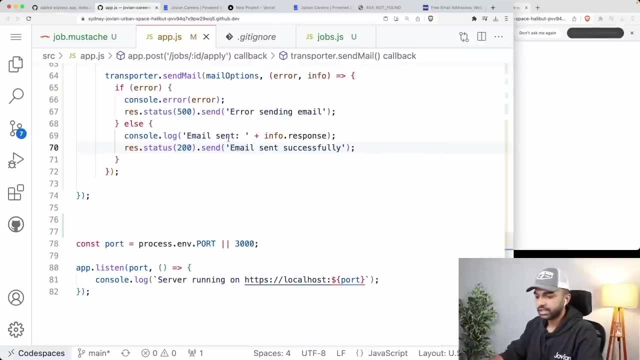 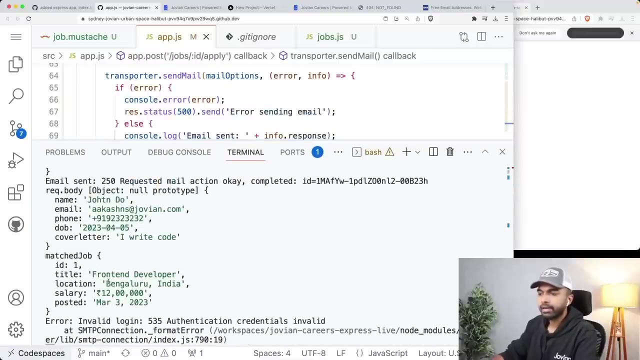 And I try to send it now you'll see that it faces an error in sending the email. and what is the error? Well, I can actually look up the error here. So if I just check the terminal and you can see that it says that I got the data, I matched. 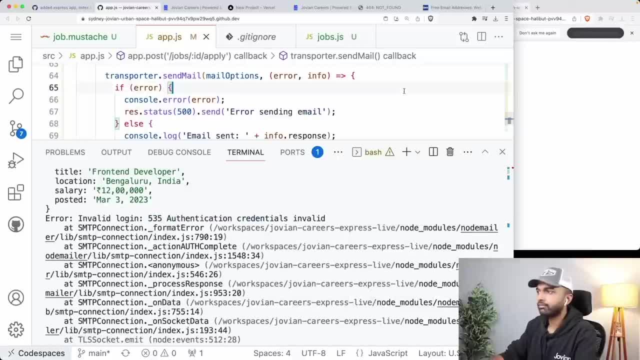 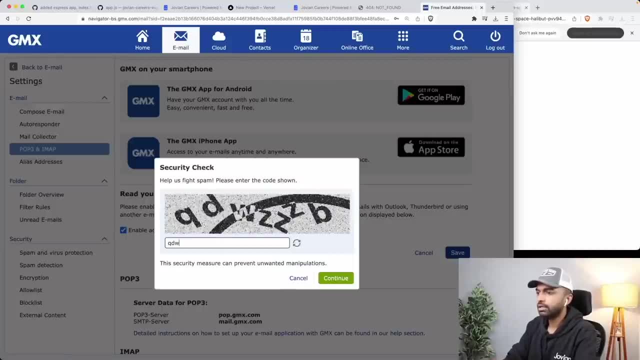 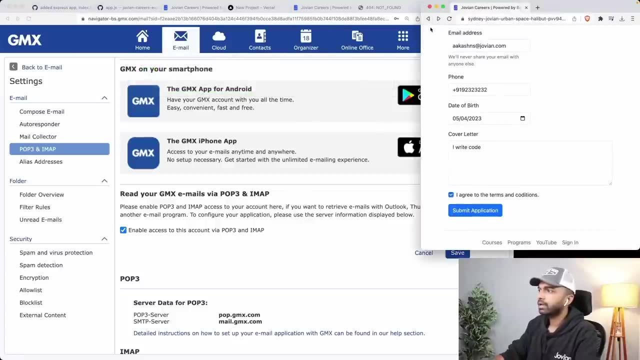 a job, but invalid login authentication credentials. Okay, Okay, So I can see that the credentials invalid, All right, But I turn this on again and save it and fill out this CAPTCHA- Q, D, W, Z, Z, Z, B- and continue, And now I try to submit this again. 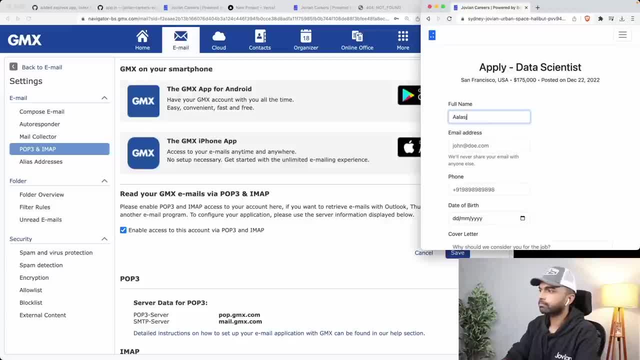 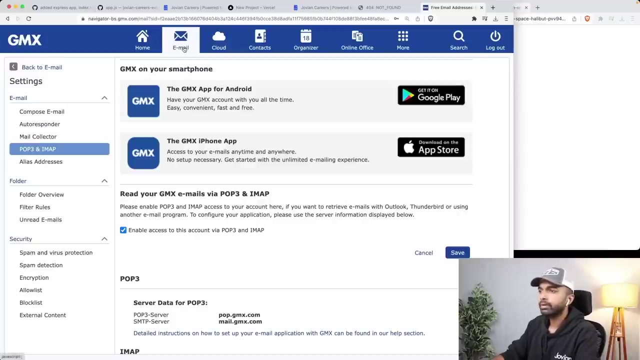 Let me try a different job this time, maybe data scientist- And let us put in a date of birth here And let's click submit, And this time the email should be sent successfully. Okay, I can come back here and check the email. 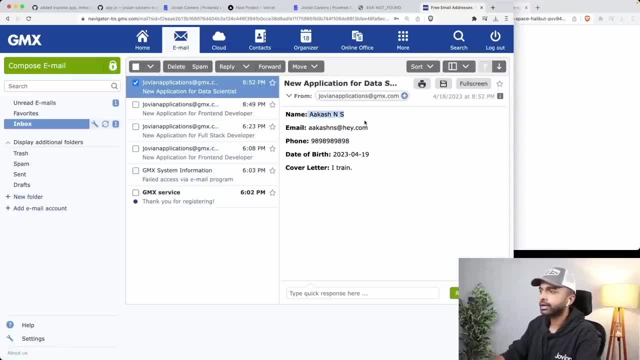 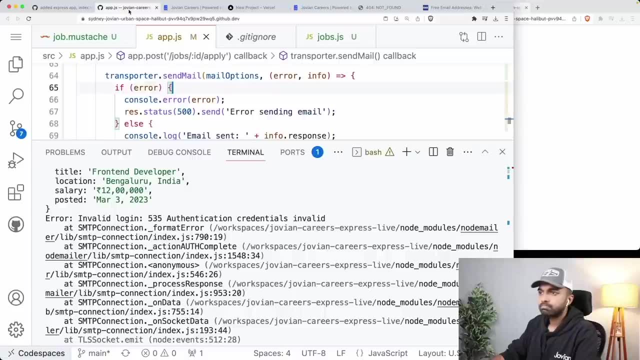 And let's see back to email and you can see there's a new application for data scientists. our caution is at haycom, such and such, And the cover letter simply says: I train. Okay, So nice. I think with that we've basically implemented what we were looking to implement. 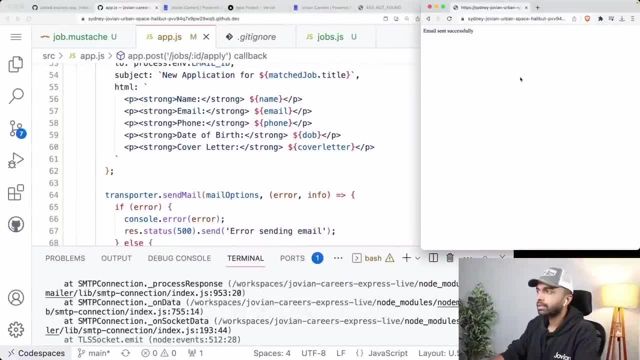 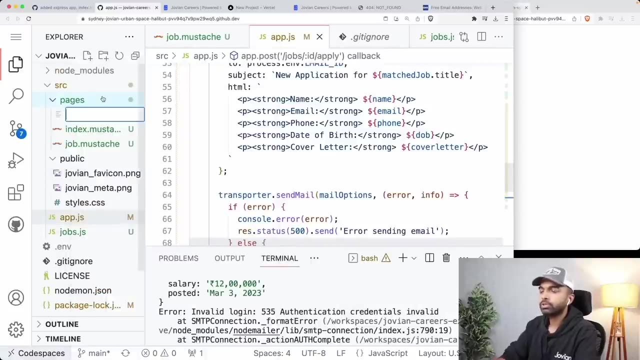 Okay, We've implemented the page here as well. Now, of course, this is not how we should show it. ideally, we should create a nice page saying your application has been received. Maybe let's try to do that as well. Let me go in here and let me say: create a new mustache template called applied dot mustache. 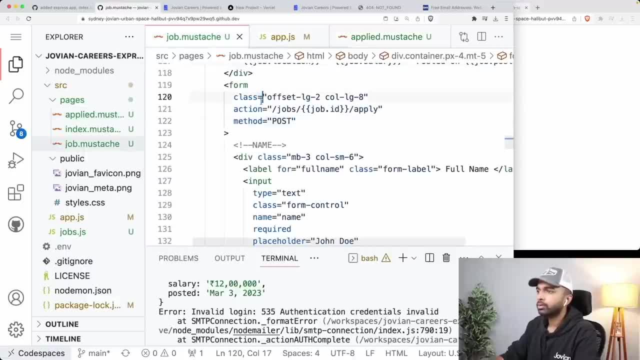 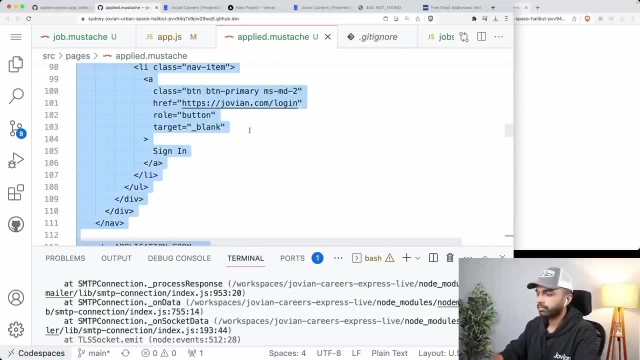 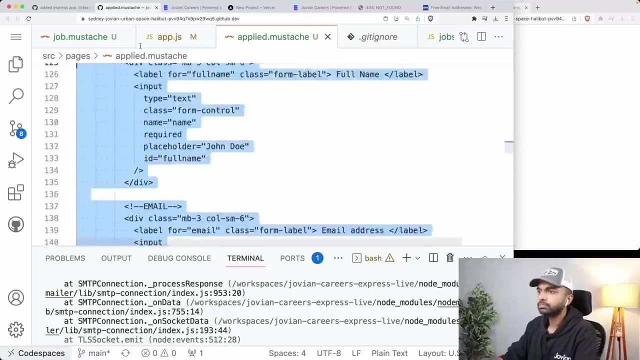 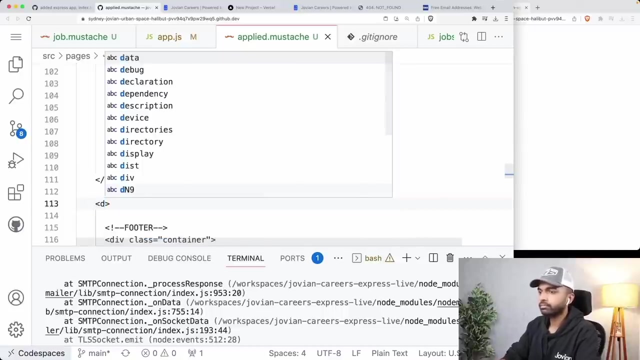 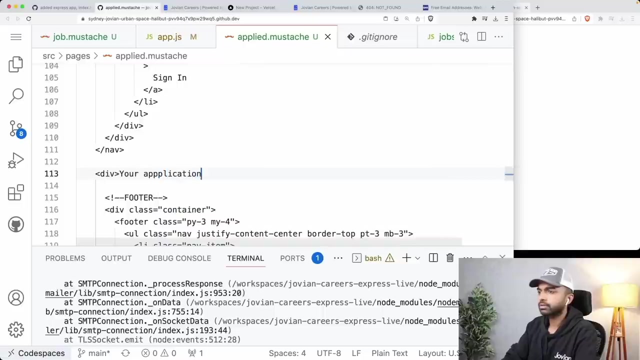 Okay, And let me go into my job. dot mustache. copy over everything from your into applied dot mustache. Yeah, and let me get rid of the form here. probably don't need the form. Let me simply say in a div: your application has been received. 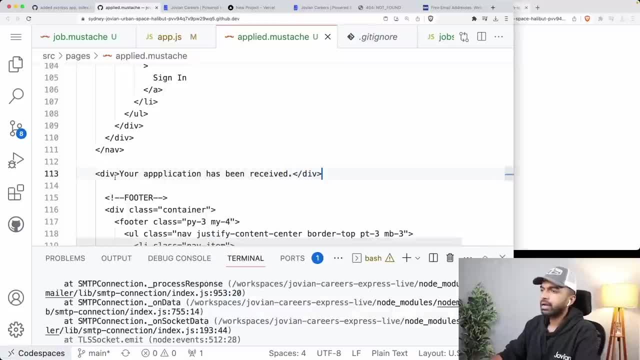 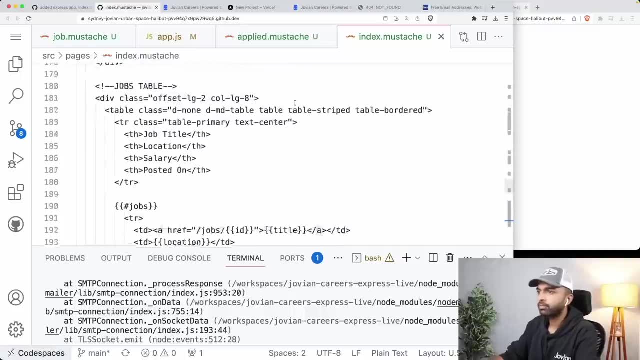 All right, I'll make it look slightly nicer. Okay, So let's see What can I do here. Well, let me go into index dot mustache. Let me get some styles from my description section, just so that it looks slightly nicer. 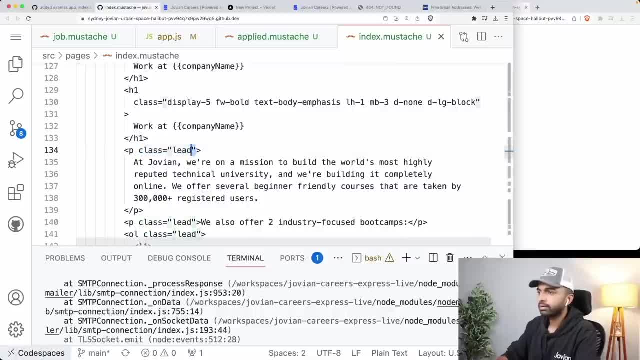 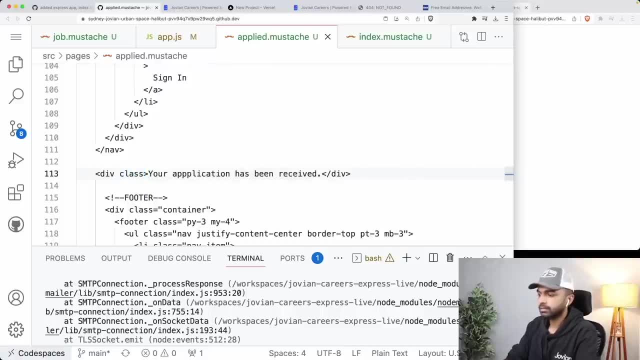 Okay, class lead. This looks good, So let me get that class lead in here. Applied dot mustache. Let me give this class container and lead, All right, Okay, so let's try this again. I click Submit application. Oh, let's also render this template. 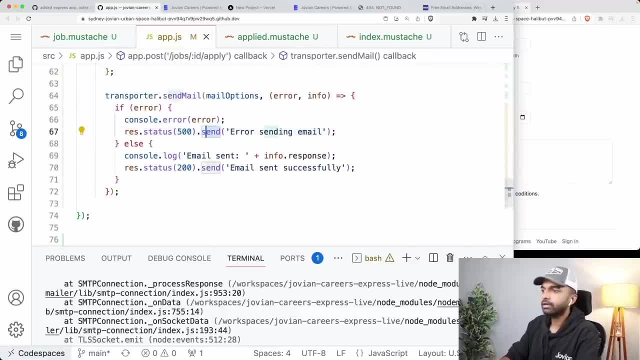 So instead of saying dot send, I can say dot render And I can simply give it the name of the template I want to render and the name is simply applied. And now, if I click Submit application, it still says email sent. it should probably. 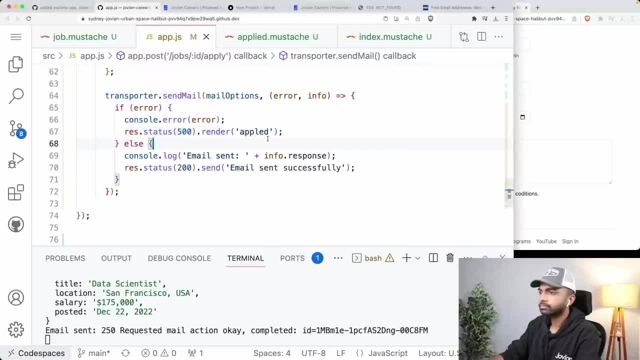 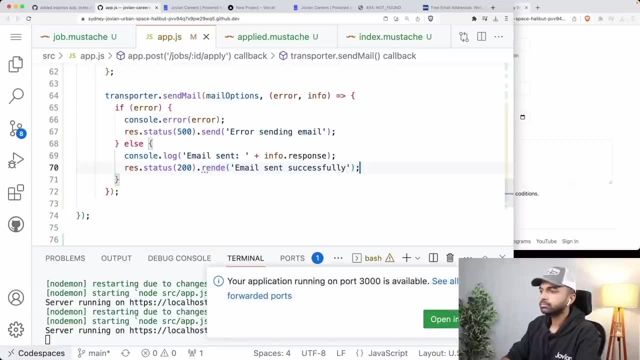 reload. Oh, sorry, I should not render this one, I should render in the other case. So dot render, Okay. So I can say dot send applied And now let's click Submit. You can see that the email has been sent and it also says your application has been. 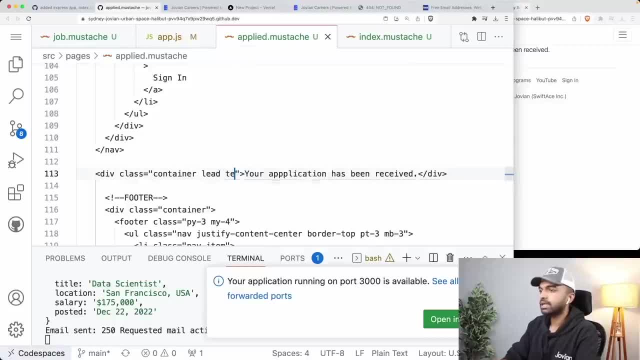 received, And of course I can make a few changes here. I can maybe say text center and I can say mt5. And it also say maybe mb5. So that this is slightly nicer. So let me go into text center. 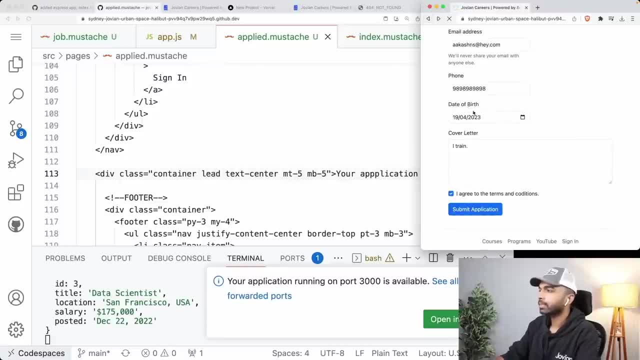 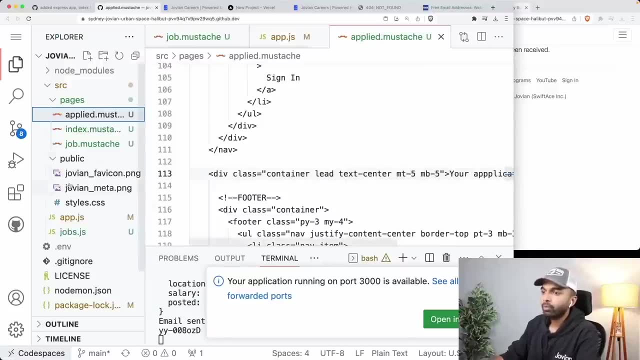 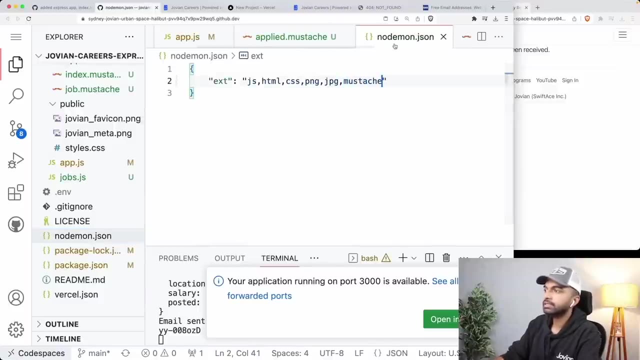 So let me go back here, let me click Submit application again, I'll have to restart something, probably. oh, I see what's happening. So we actually want to reload the server even when a moustache file is changed. So M U S, T, A, C, H E. I'm adding this setting inside nodemonjson so that whenever I change, 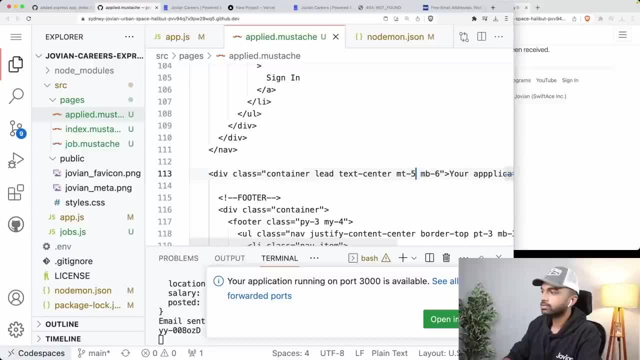 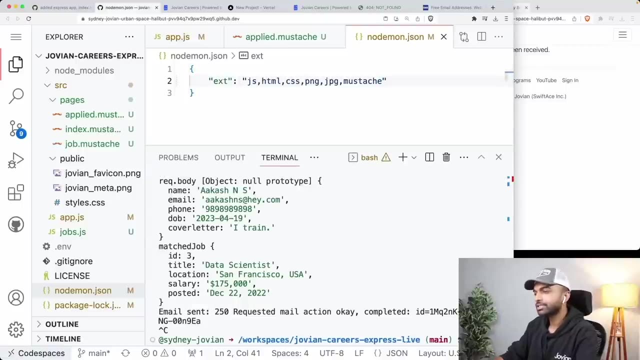 a moustache file that automatically reloads the server as well. Let me make these mt6 and mb6.. Let me go back and submit application. Okay, I need to restart nodemon as well. When you change nodemonjson, you need to restart nodemon, or you could just do. you could. 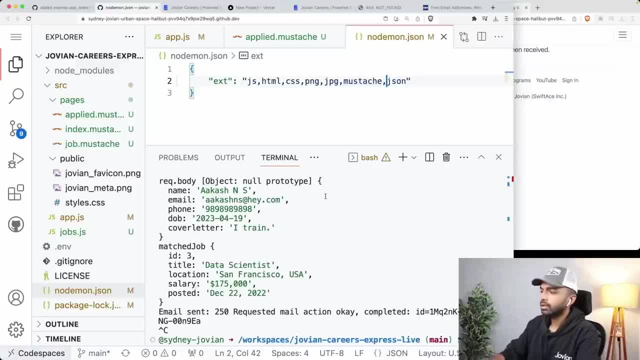 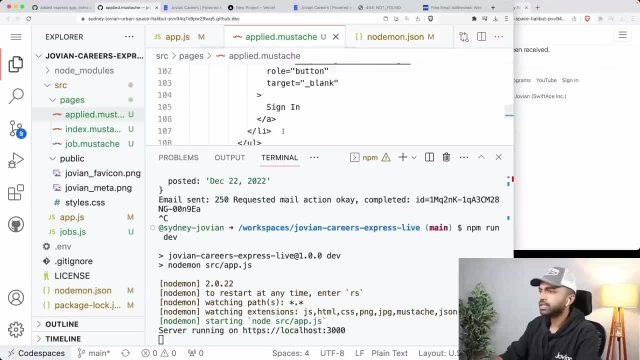 add JSON as another file that it watches for as well. Okay, But npm. oops, let's run it again. npm, run dev, And let me just fix the spelling here. I think there is a small fix it. we have three P's here. 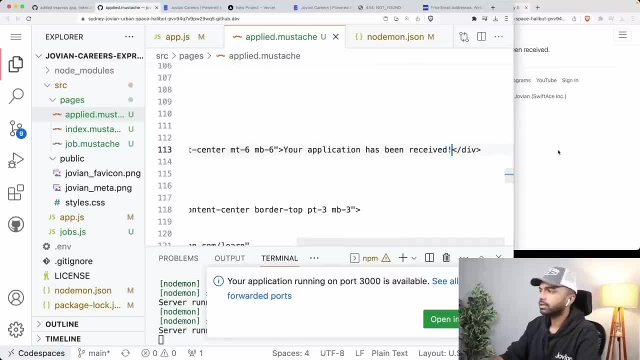 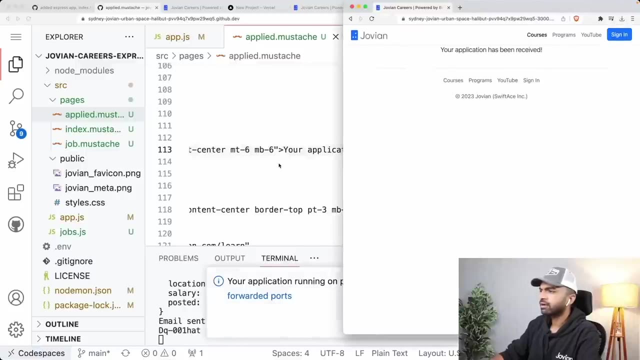 Let's do that. Let's do that. Let's put this in here: quotations. Let's go back and let's click Submit application and it says your application has been received. Okay, perfect. So with that, we have implemented, we should have a, probably a top margin as well. 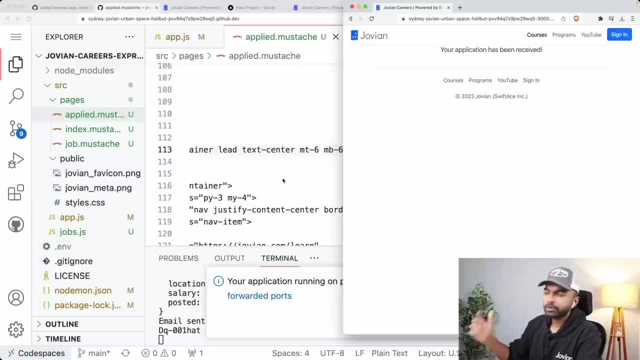 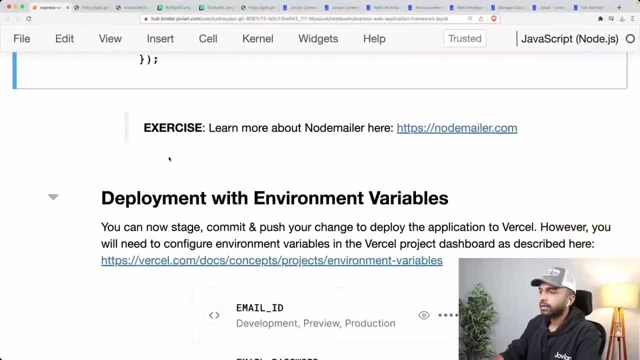 It's not showing up just yet, But you can always figure that out. small styling changes- I'll leave that to you as something to do. But with that we've implemented a nice applied page as well. That's nice Now. So we want to actually deploy this. 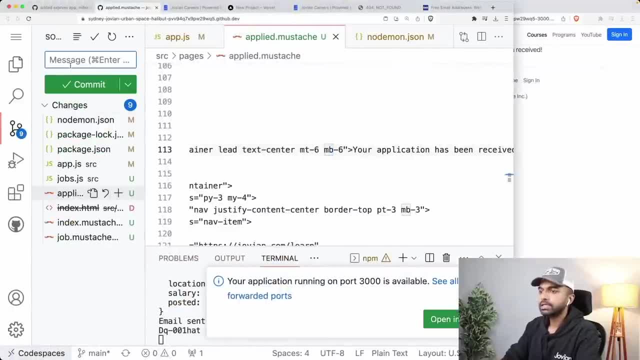 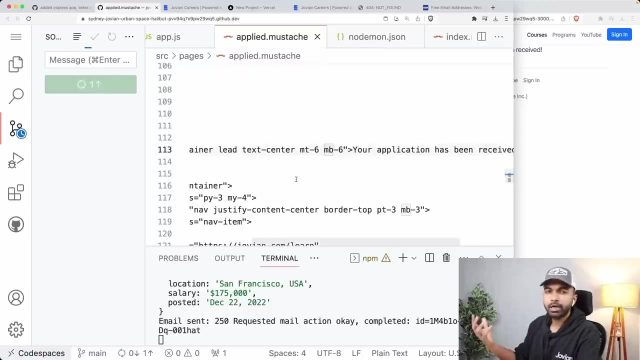 So for us to deploy this, of course we can go in here and we can say: added templates and dynamic pages and click commit And let's send this. that's going to go to GitHub and that is going to automatically deploy to Vercel. 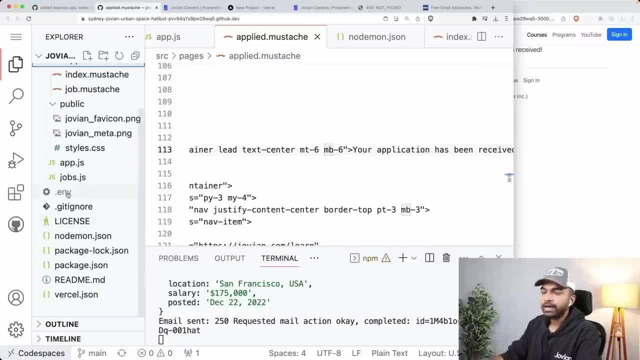 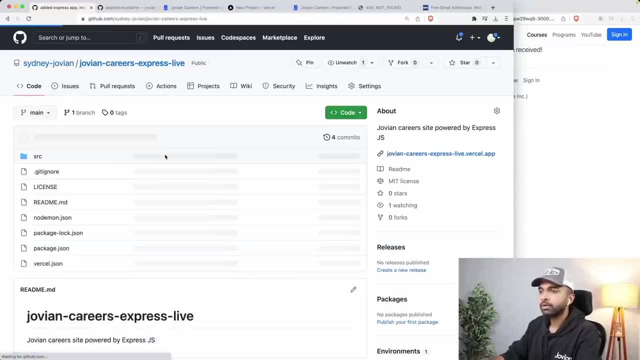 However, remember that our dot env file is not, is not going to get committed to the GitHubreport. Okay, Okay, So let's go back to my GitHub repository. which means, if I look back at my GitHub repository over here, that is going to contain everything, but it's not going to contain the dot env file. 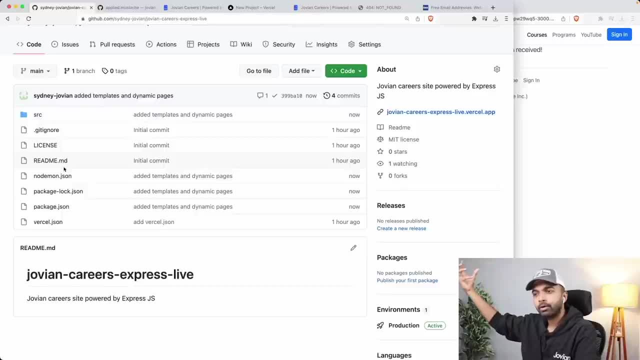 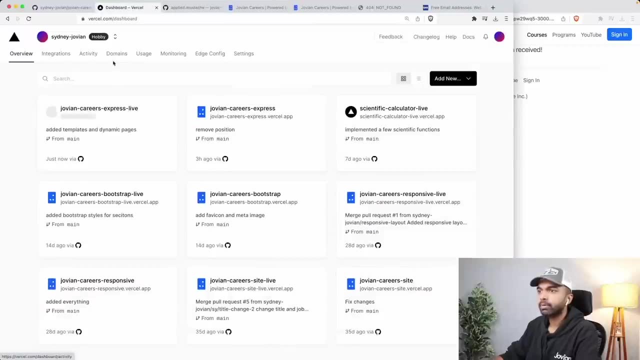 So when Vercel picks up all of this code and tries to deploy it to the cloud, Vercel doesn't have my credentials. So I need to give Vercel my credentials. Let's go back here into the project Jovian Express careers live. 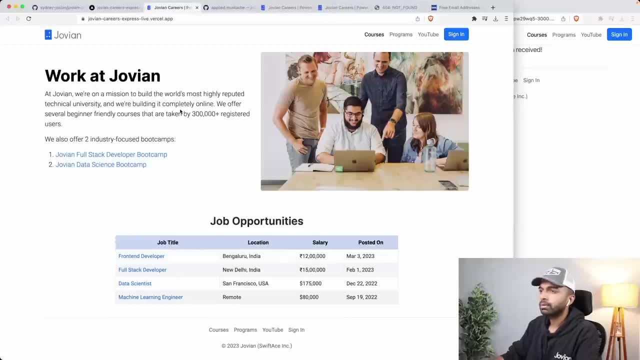 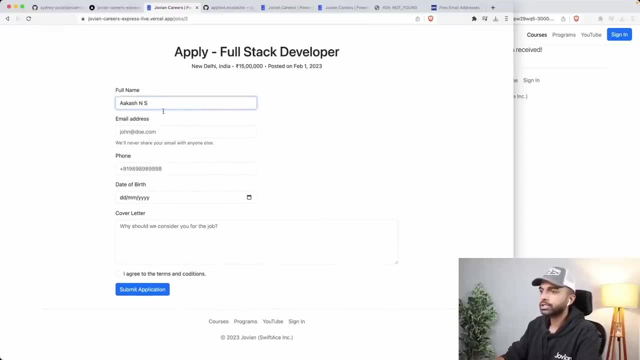 And let us actually see it in action. Okay, work at Jovian, This is all well and good, full stack developer- All right. So let me put in some information here. our caution is a ad at bcom, Something like that. 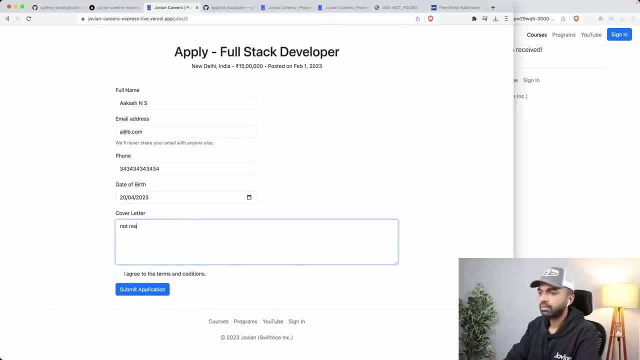 And let me put that in your cover letter: Not ready. And let me click Submit application And we're going to get into this error: error sending email: obviously because Vercel doesn't know the email and password that we need to have right. 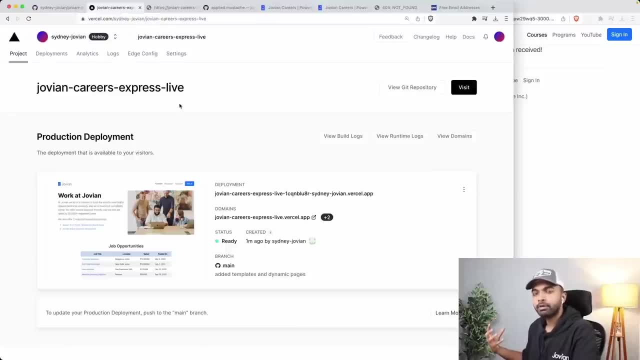 So that is where, just like you have environment variables in a dot env file for local development, Vercel has a settings tab And inside of that we have a dot env file And inside of that you can specify some environment variables. 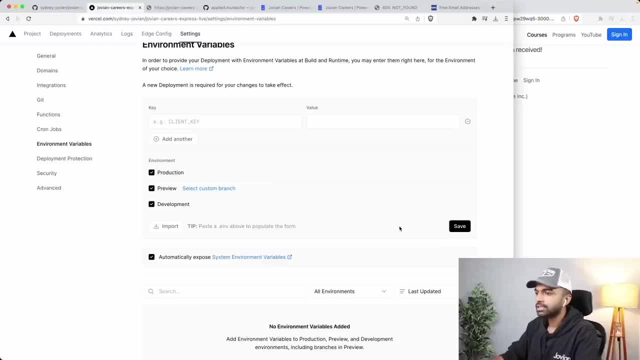 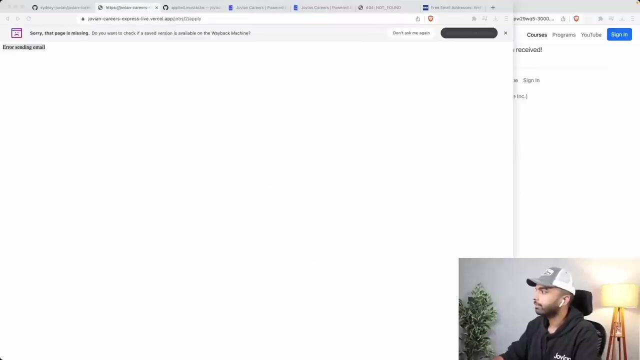 Okay, So here you need to add in a couple of environment variables, And I believe I can probably just face to the contents of an environment variable file. Yeah, but I just want to do that securely. So I'm going to go in here and paste my environment variables to my email ID. 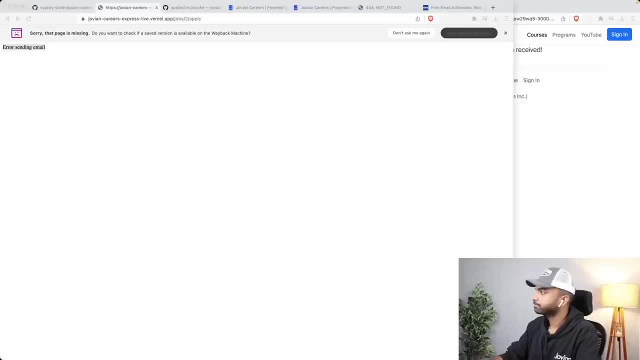 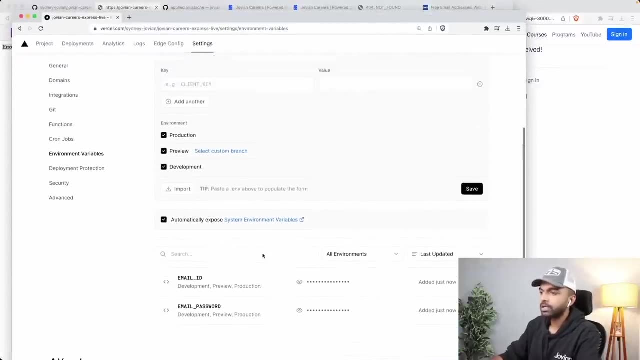 Yeah, and I've added them, And now I'm going to just save them. Yeah, And now they have been added. So they've been added below. I've added my email ID, I've added my email password and these are stored securely on. 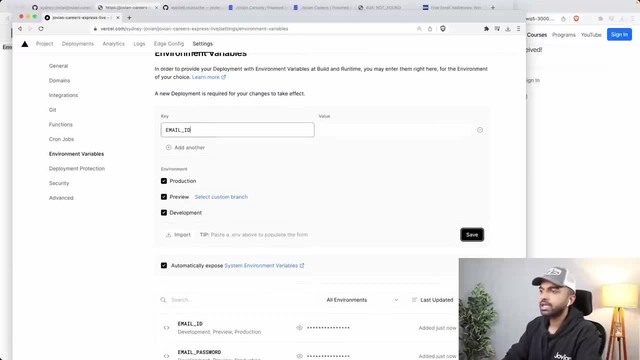 Vercel And I can add. so the way I basically added this was to say email underscore ID and whatever at whatevercom And I click Save And that is how these got added. Okay, So now the environment variable, my email ID and password, have been added into Vercel. 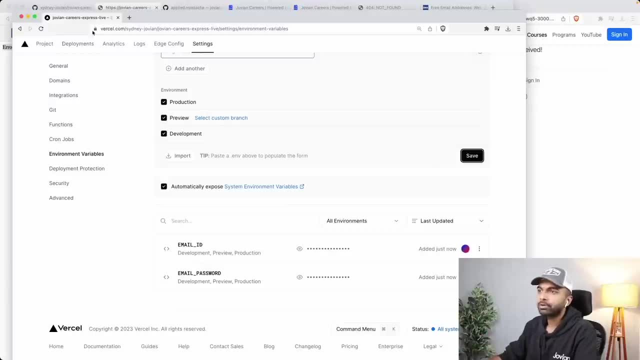 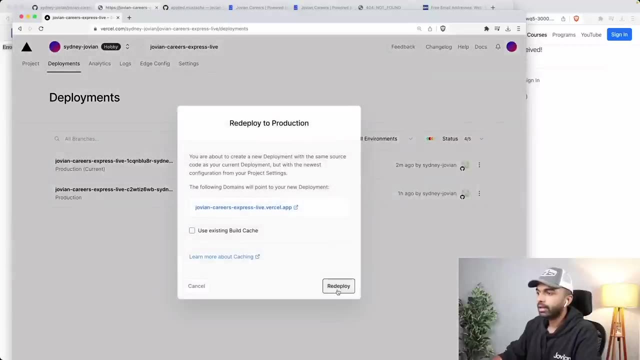 and it is going to populate them into process dot env And that is going to then get picked up. but I just need to do one more deployment to actually send it. So let me just do redeploy, and redeploy is going to take a second, is going to pick up. 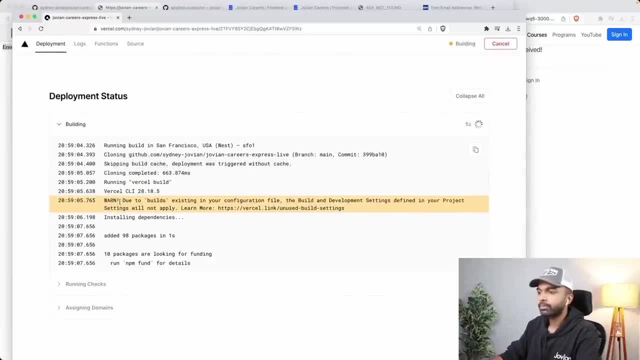 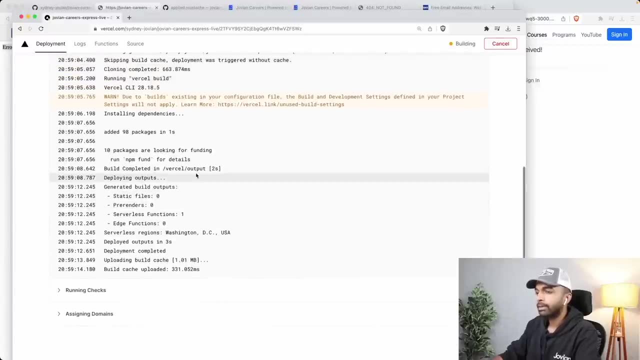 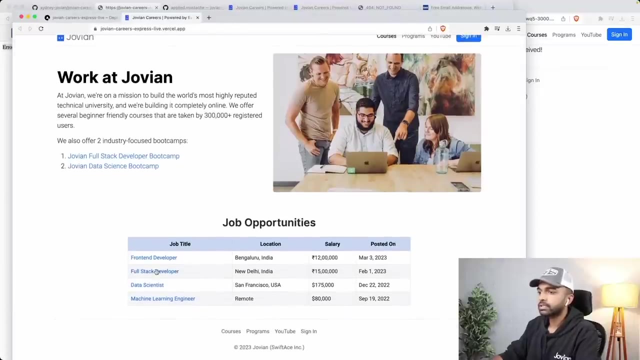 all the environment variables as well this time, And it is going to redeploy this Vercel is going to redeploy the package or the application, And now let's go back in here. Let's try again. Okay, full stack developer role. 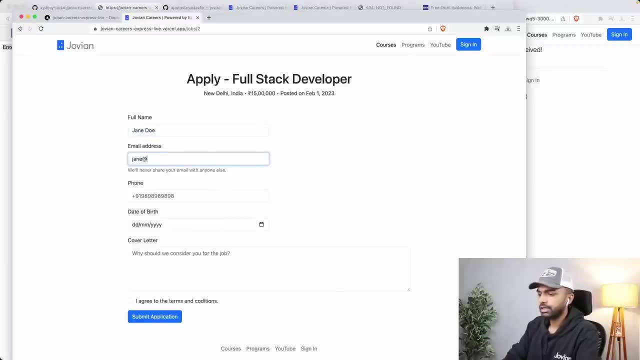 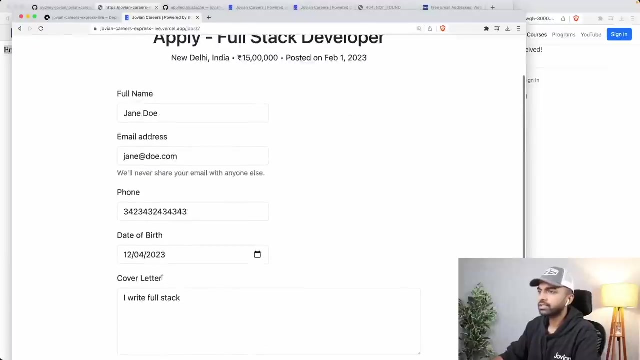 Let's see Jane Doe Jane at doorcom Like that, And let us just fill that out here So I can zoom this in for you. But you have simply filled out for the full stack developer. I've simply filled out the application and click Submit. 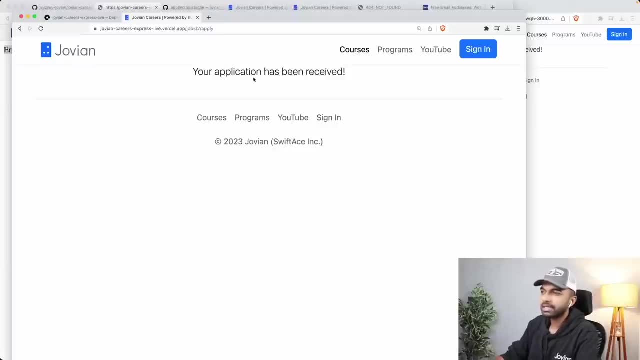 And this time it says: your application has been received. right, we can add some space above it, But I guess this is fine. I can also then go into gmxcom, And this time it says: your application has been received. 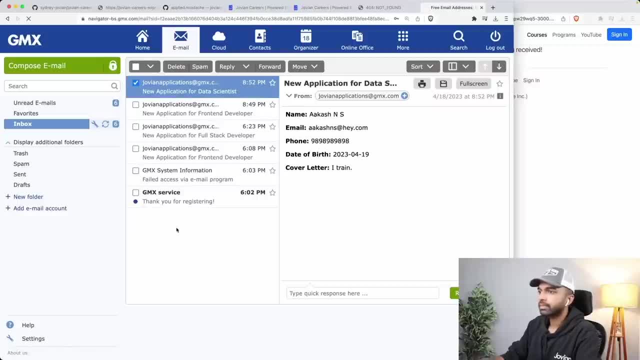 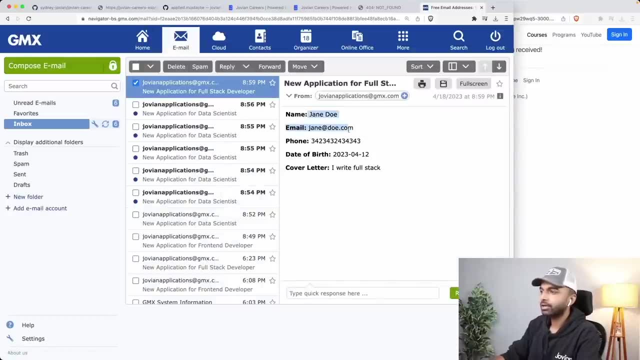 And we can add some space above it. But I guess this is fine And let's see, Let's just reload this page. This is a very old email service, So you can clearly see that you have to reload things and all. but yeah, Jane, Doe, Jane at. 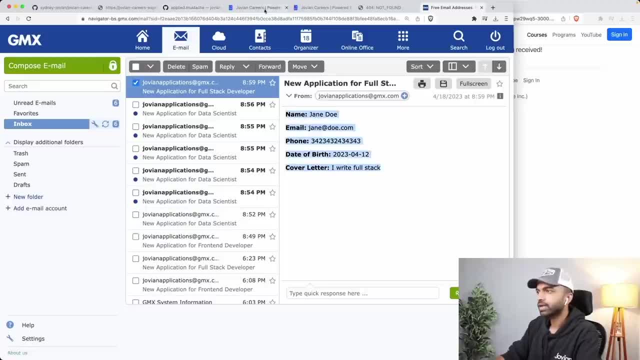 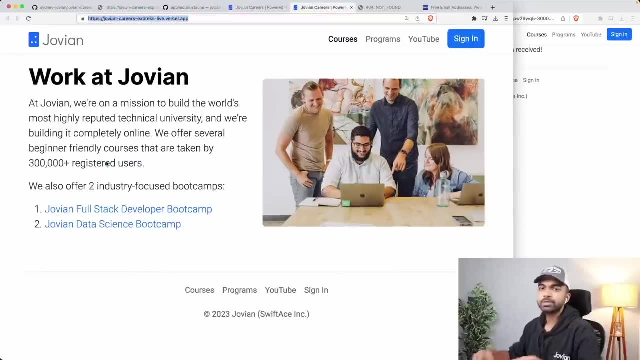 doorcom phone. date of birth, cover letter: Perfect, And with that we are more or less done. So now we have created our website, which anybody can use, And this is a website that, honestly, at this point we can probably deploy as our careers. 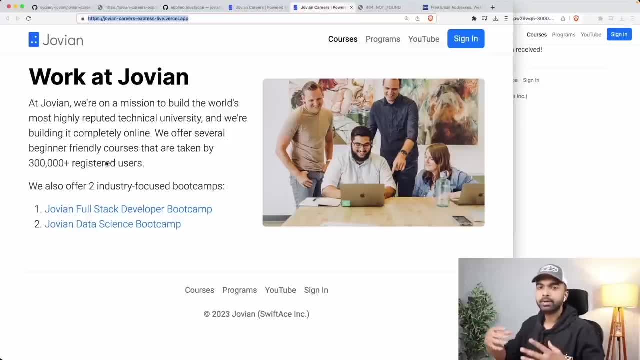 website. maybe just change this image to an image of our team, maybe just update the roles that we have in our in the repository and then deploy it. But the next step here would be maybe adding some sort of a login system, maybe storing the data in a database and maybe allowing applications also to be stored in the database. 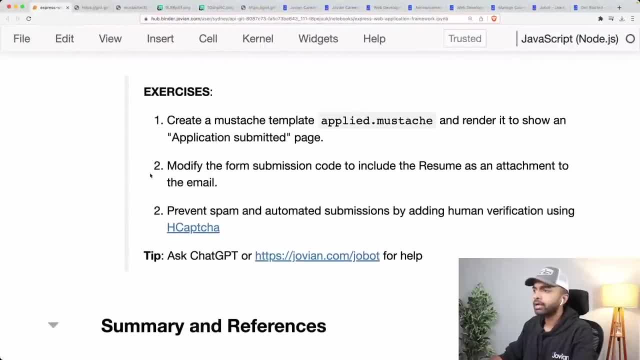 and so on, But there's a lot you can do here. Now here are a few exercises for you: create a mustache, template applied or mustache. we've already done this, But how about? apart from saying your application has been submitted, you also show what is. 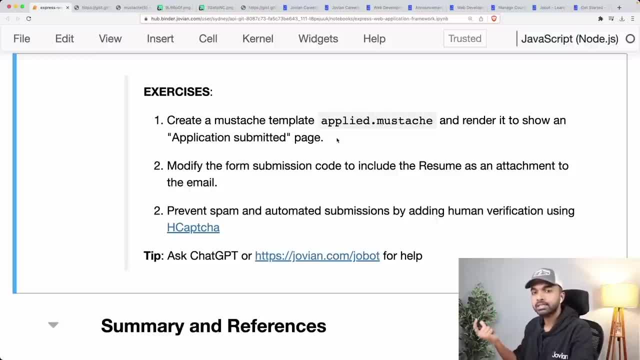 all the data that the user has filled out. Remember you still have. you can pass a variable. You can pass a variable, The. you can pass a request body, maybe as the application data, into the template and you can populate the template and show all the data there. 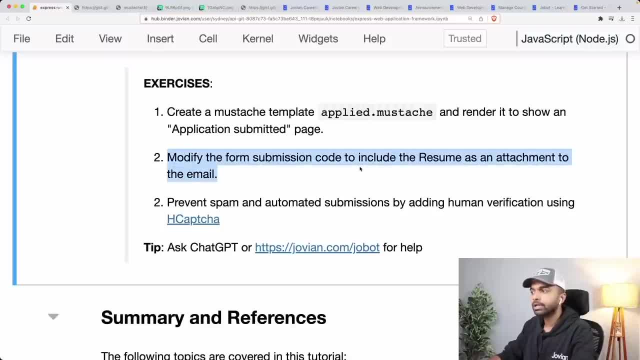 Or what you can try, modifying the form submission to include the resume as an attachment to the email. So what happens here is you have to use a encryption or encoding type called multi part form data, And for that you will have to use not body parser but something called murder. 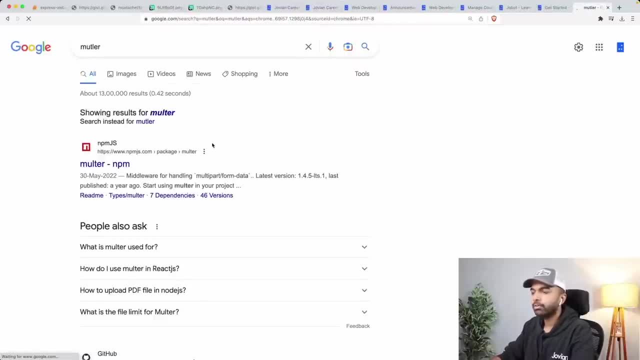 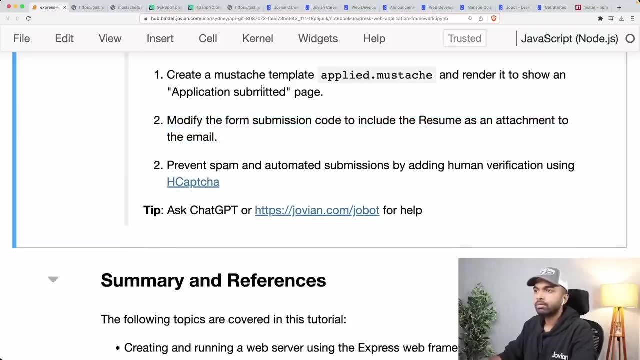 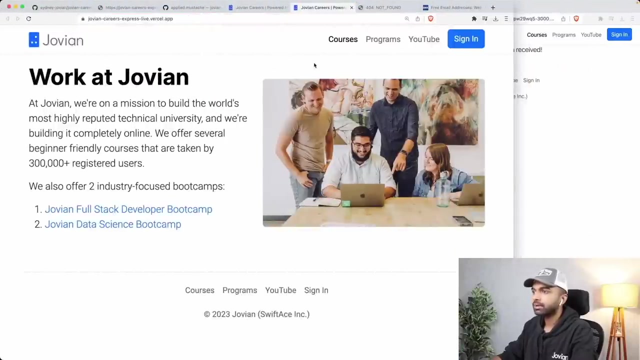 Okay, So murder is a middleware for handling multi part form data in Express. All right, so I'll let you check that out as well. Here is another thing you can try to do. now. what might happen is somebody can create a quick script that can open up the page, or maybe like some kind of a web scraping script. 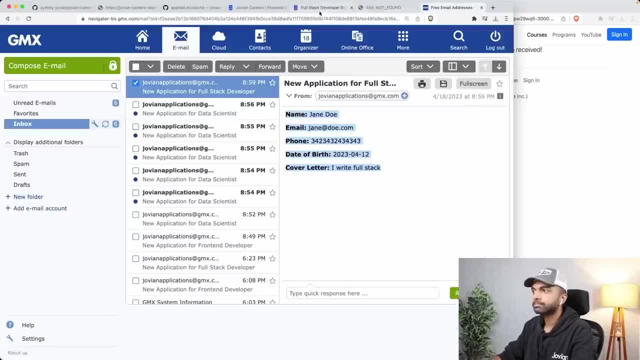 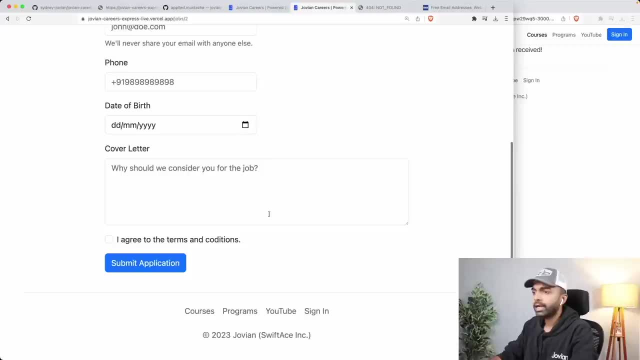 that can open up the page and then just fill out hundreds of applications. and then, yeah, fill out hundreds of applications. Let me reload that. your fill out hundreds of applications by simply automating this or clicking the Submit button again and again and again, and that will lead to hundreds. 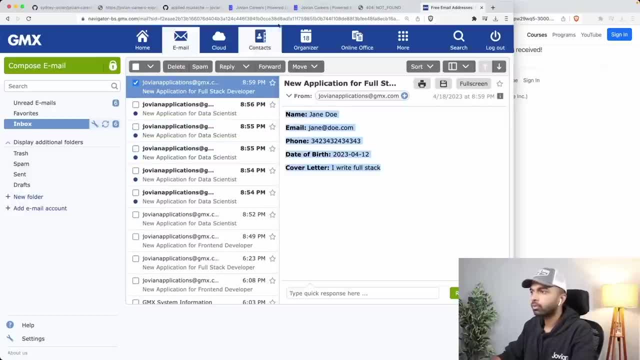 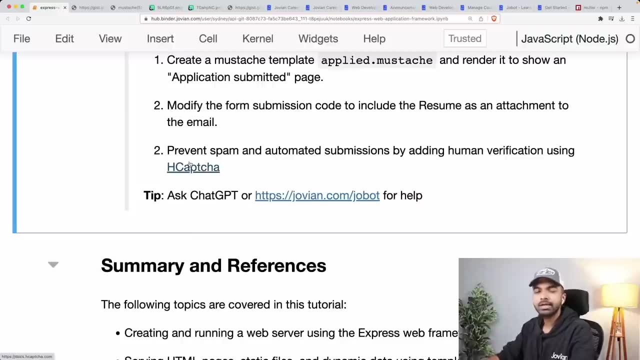 of email over here. So we want to avoid that. we definitely don't want hundreds of emails, And for that what you can do is use some kind of a captcha that you see that thing where they ask you to select traffic signs and all. it's actually very easy to add. 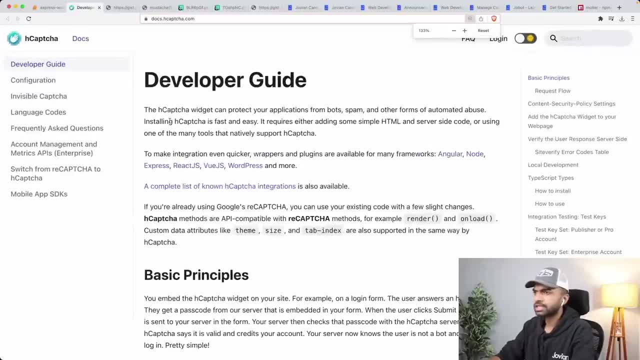 And one one captcha system that you can use, which is actually easier to use in Google's recapture, is the edge capture system. Okay, So what you'll have to do is you'll have to go in and log in here and you'll have to generate. 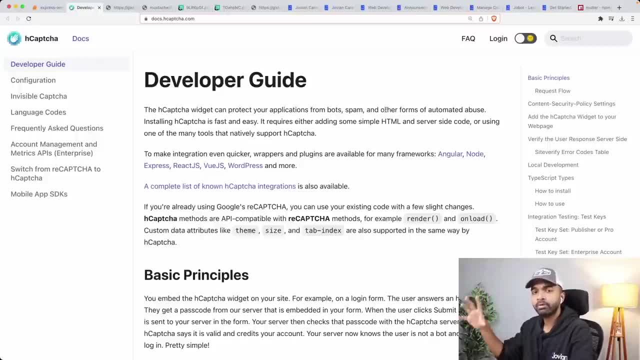 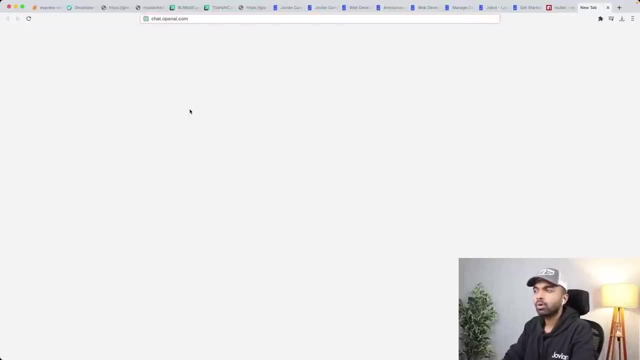 some. you'll have to put some code into the indexhtml file or whatever HTML you're sending to the browser. You'll have to put some code on the server, and you will have to then just verify that it works properly. Okay, Now, one good way to do some of these things is to maybe just go on, let's say on jobart. 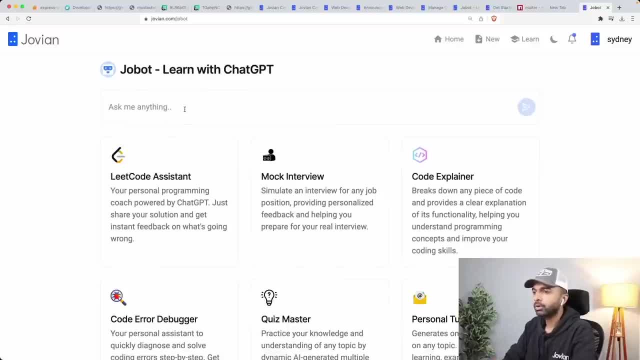 So joviancom slash jobart and you can ask jobart, show me an example of how to add spam protection. Okay, Okay, Okay, Okay. So you can see that you can add some captcha in an express JS application, Okay. 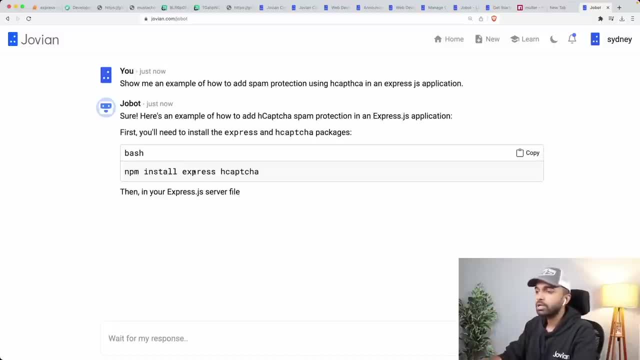 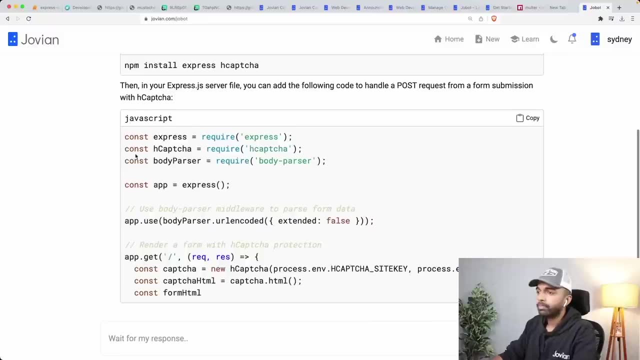 And just like that, jobart should be able to tell us exactly what we need to do. So first you need to install the NPM install edge capture package. Then, inside your express server file, you need to require the edge capture package. And then what you need to do is a couple of things. 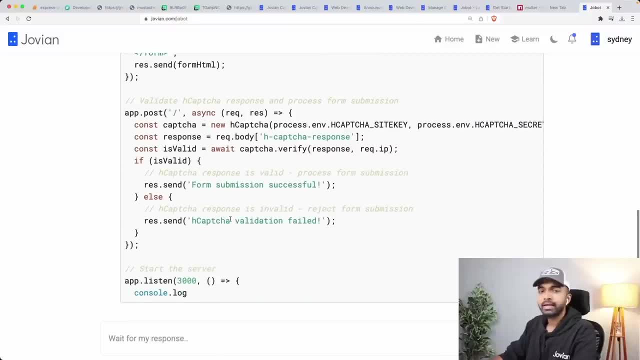 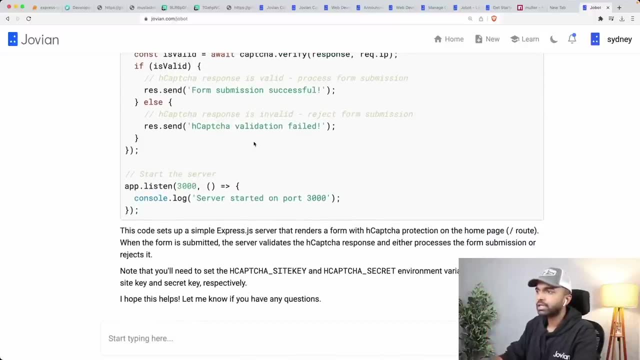 One. you need to create some captcha HTML and send that into your file template And then, second, you need to maybe verify the captcha response using captcha dot verify from the body. You can get this. get this edge: capture response and verify it. 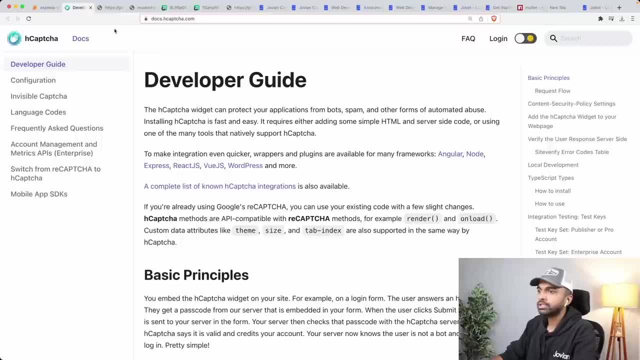 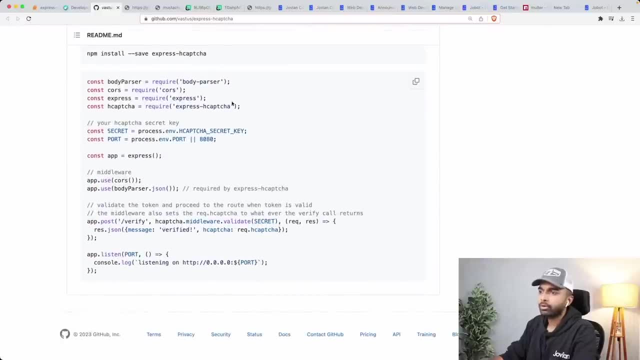 Okay, And that's it Right. Or you can also look at the documentation. So the documentation: there is some documentation for express JS and here you can check it's example and it says something about how you do it. So there are many ways to do it. 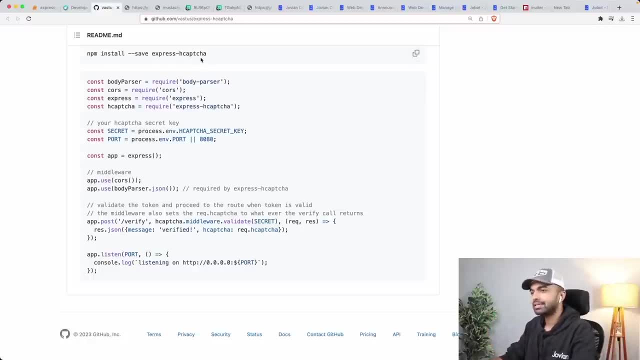 Just look it up. This is a very common use case that people do, Okay, Okay, There is a pattern from now going forward that it is impossible for us to just learn or teach or remember all of the various possible things that you can do. 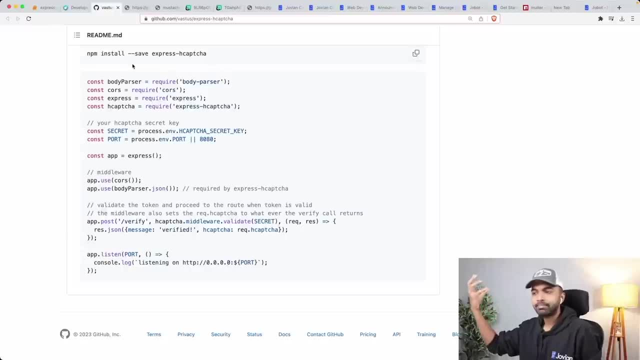 From this point on, what you need to do is figure out what you need. For example, I need a captcha. then search online, maybe study the documentation, maybe use chat, GPT or job, or look at somebody's blog post. understand the code that is there. 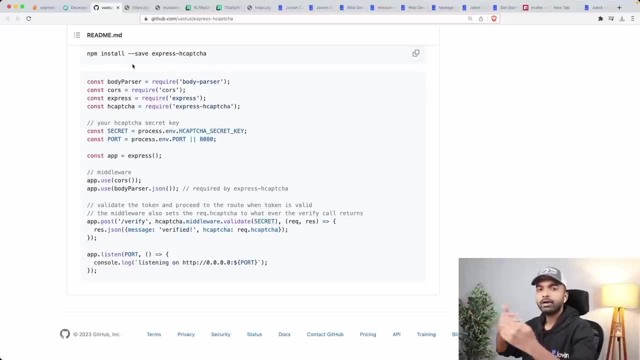 Bring that code into your project, because that code is never going to be directly copy pasteable. Bring that code into your project, Test it out And if something goes wrong, check the documentation. repeat the process again, debug things, test it out. 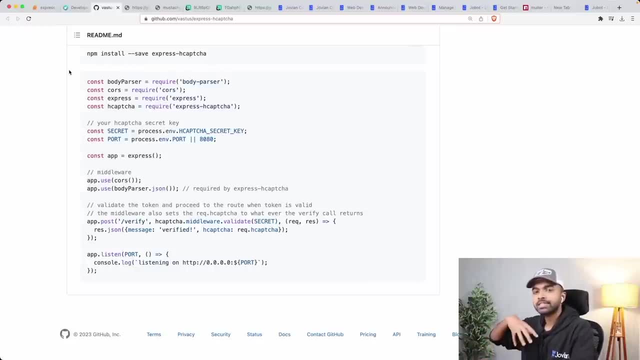 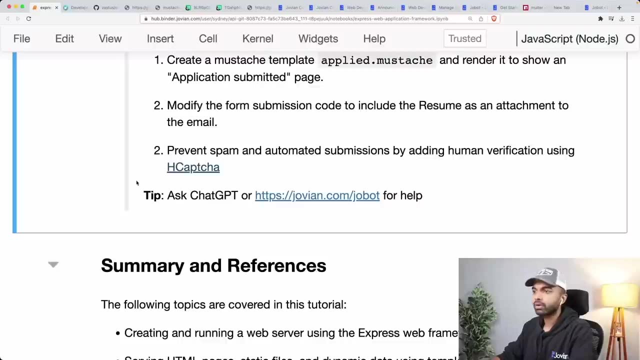 And once it works, you're good to go Right, And with that, you now have access to potentially thousands of libraries and thousands of features that you can easily incorporate into your web applications. All right, So I'll allow you to do that. 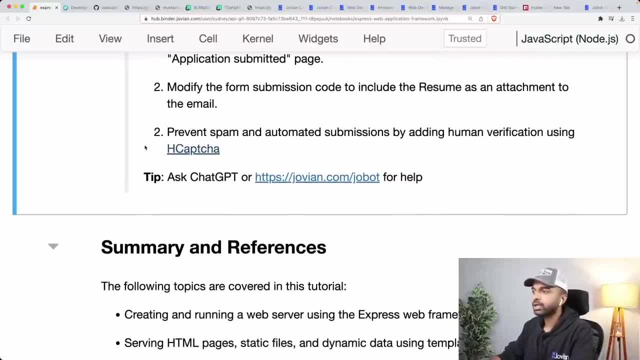 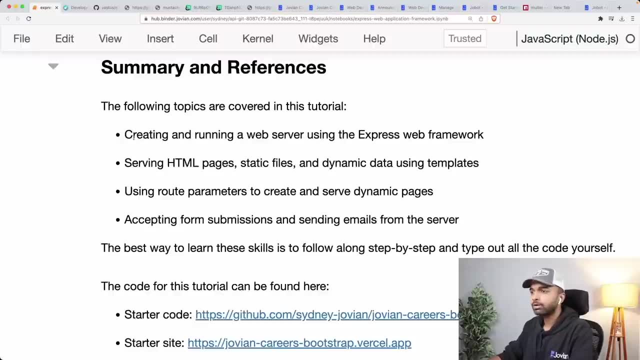 Modify the song, modify, prevent spam and automated submissions by adding human verification using edge capture and use chat, GPT or job bot for help. Okay, So here's what we did today. We created a and ran a web server using the express web framework. really simple, just. 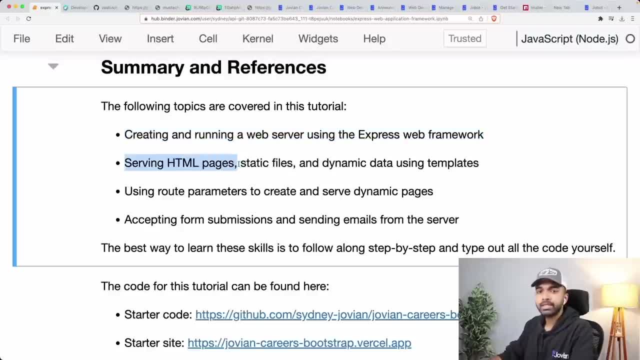 a few lines of code. We saw how to serve HTML pages and we saw how to serve a static files, And then we also saw how to serve dynamic data using templates, where we use the mustache templating engine and we filled in jobs data from a list. 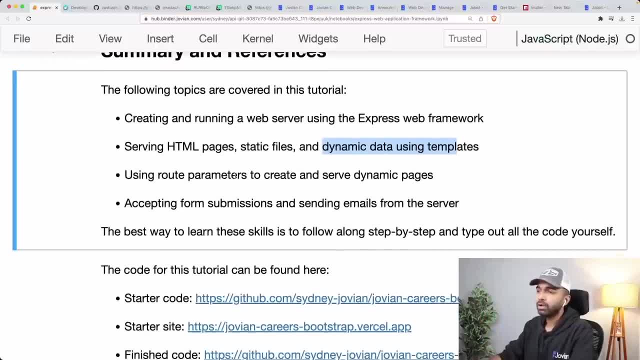 It could also have come from a database into the template. We also saw how to use route parameters to create and serve dynamic pages. So we created a job wise application Page where we showed the job title, salary, location, et cetera at the top of the page. 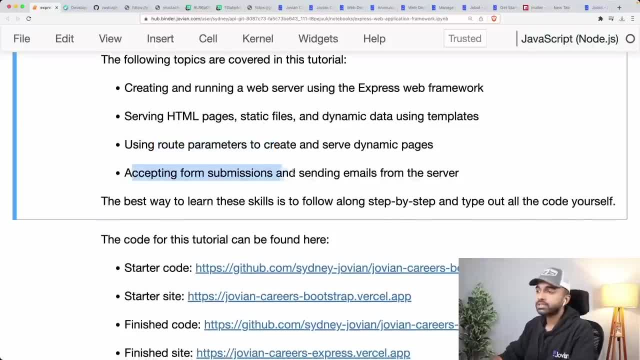 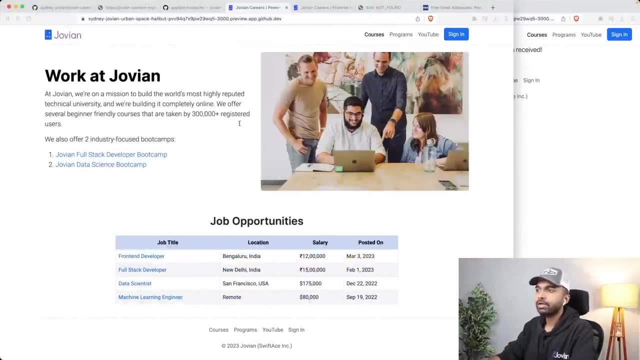 and the application form. And then we also accepted form submissions on a new route, which was a post route, where we pass the request body, We pass the content from the form that was submitted And from there we got the emails. And, by the way, if you have a doubt, how did we get to know that the form had this? 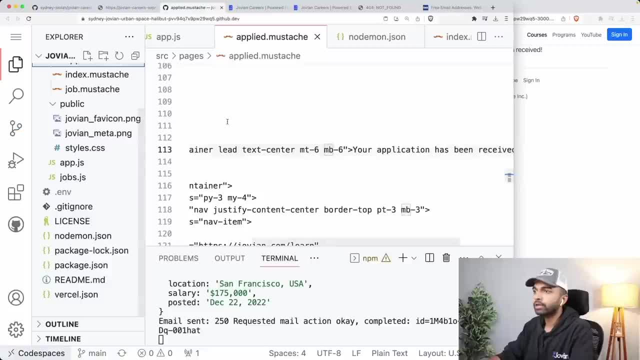 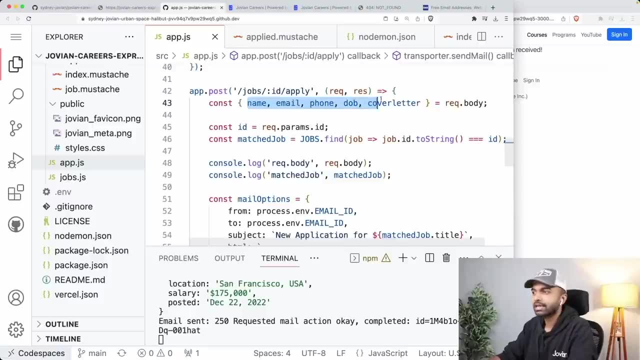 Yeah, If you have a question how we got to know that the form had had certification, Okay, We got the content. He is. So you have these things here. How did we get name, email, phone number? How do we know that these were the actual names of the keys within the form? 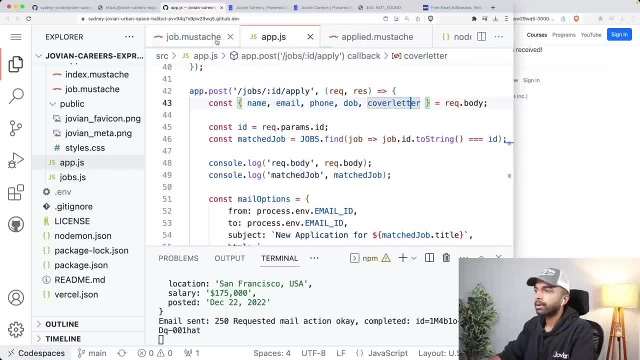 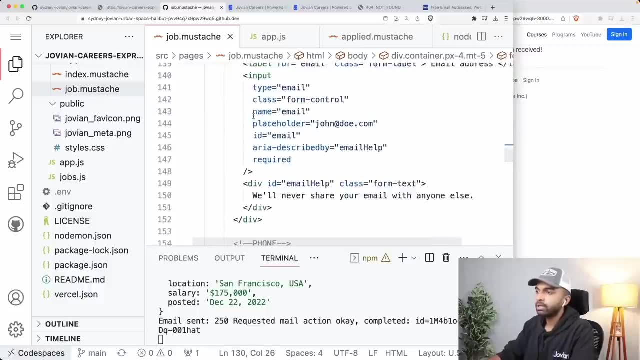 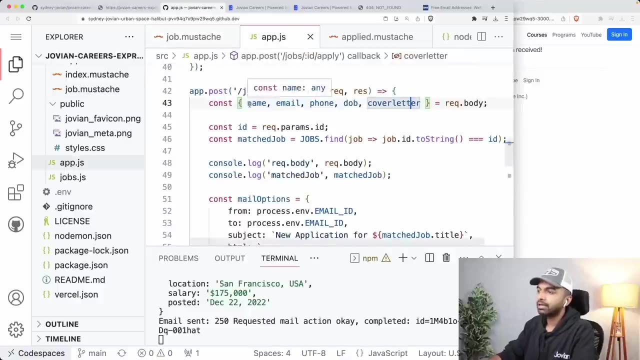 Well, that is actually present within the form itself. So if you check the form, for every input we specify the name. So name equals name, name equals email, name equals phone name equals DOB. And that's exactly what we get: your name, email, phone, DOB. and then there is that. 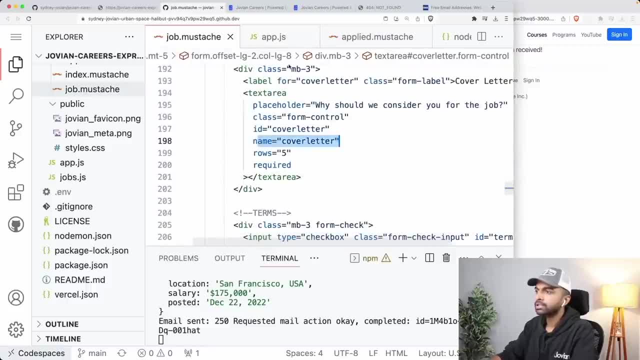 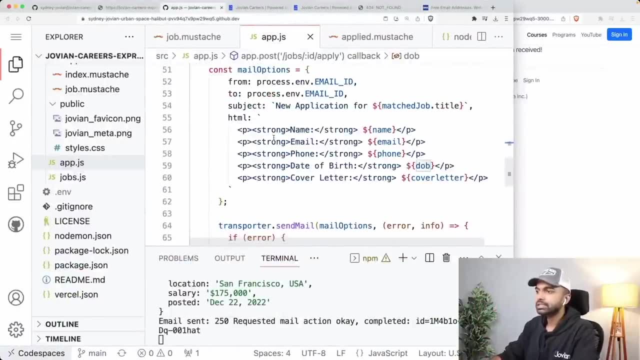 last input, which is the cover Letter. name equals cover letter And that's what we get as a variable cover letter. Okay, So we got all the data from the form and then we created this mail and we use note mailer to configure our settings. 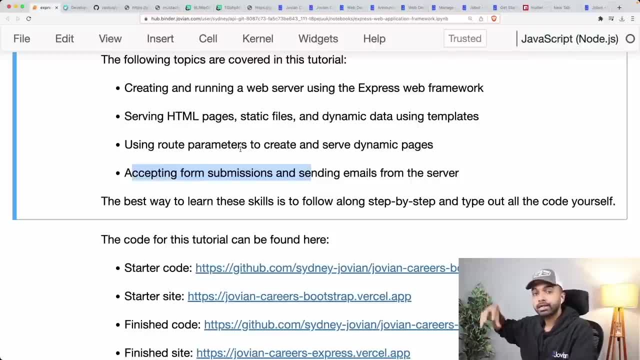 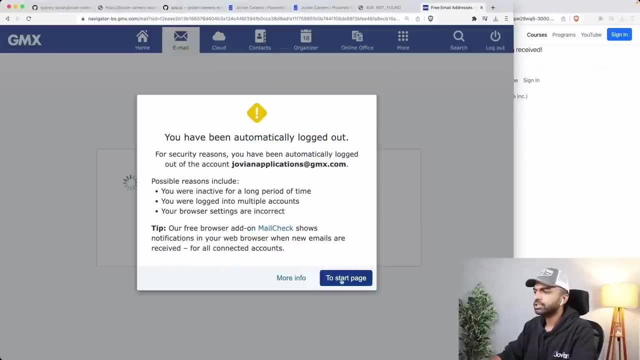 Our credentials are credentials of basic posts. Our credentials were stored securely in a dot ENV file, read in securely using the dot N library, And then we created a transport and from that transport we present an email and that email was then visible here on our GMX account. 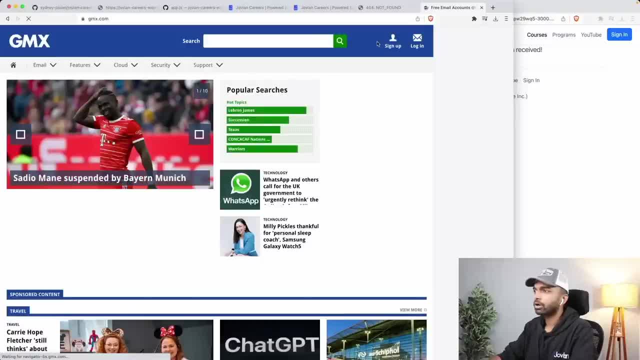 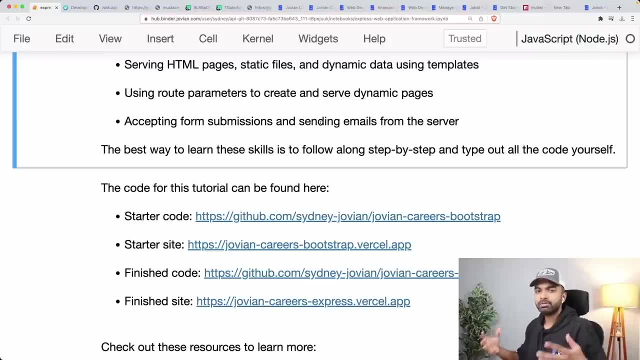 Yeah, So maybe I was just I got logged out here, but yeah, that was available on a GMX account. So that's how you build a web application, right? This is the most basic version, where we're simply using HTML, CSS, JavaScript. 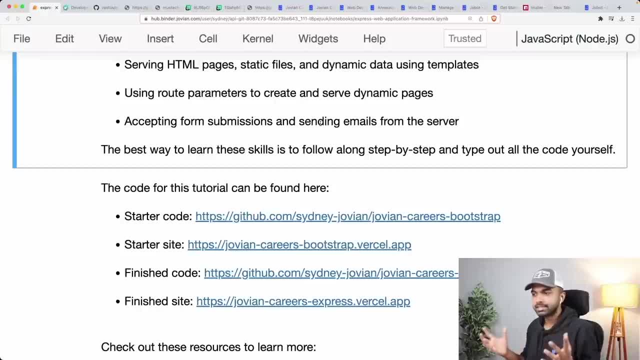 We are not using things like react et cetera, but this is the core. The core idea is going to remain the same. You have a server, some logic happens on the server. server can connect to the database, server can process requests, server can handle form data, et cetera, et cetera. 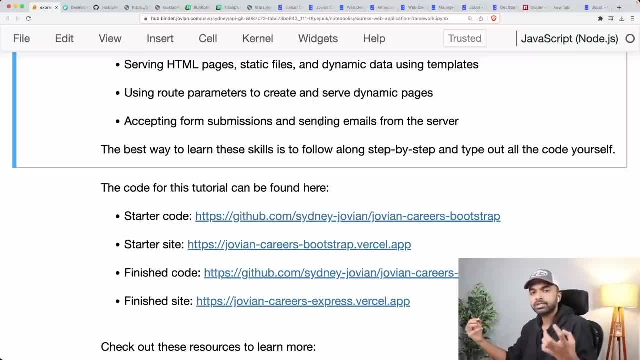 Okay, And then you send some HTML to the client and that, along with that HTML, you might have some CSS, You might have some static files, You might actually also have some JavaScript files which get executed only on the client. All right, 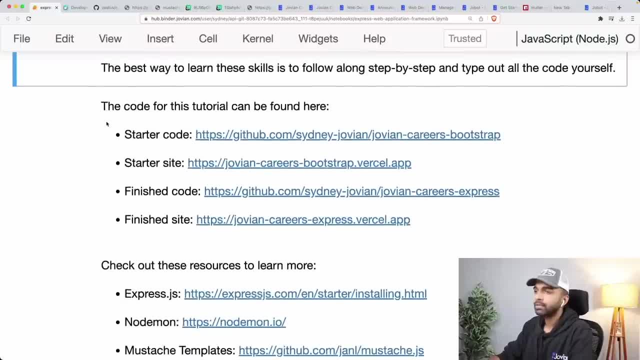 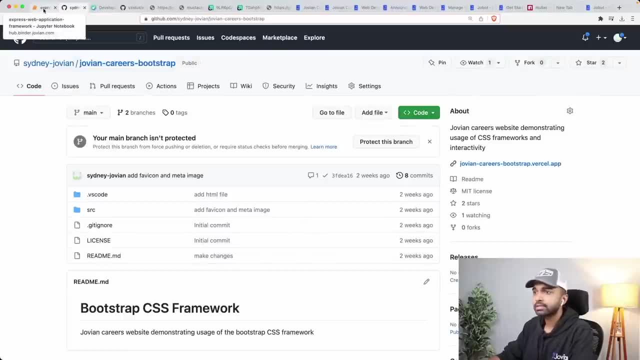 So all of that is something that you can do as well. Now the code for the tutorial can be found here. It's all open for you to see, so you can check it out, except, of course, the credentials themselves. This is the starter code and this is the finished code. 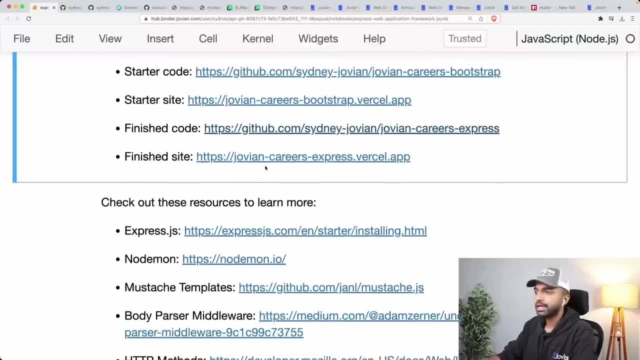 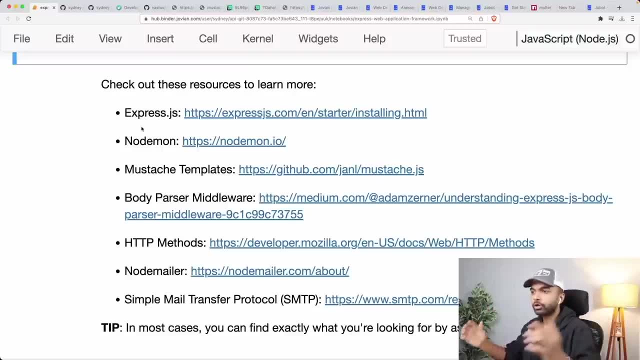 So this is all the finished code that you can look at and this is the finished site that you can check out And check out these resources. to learn more at this point, you just have to Google things or ask Jobot or ChatGPT. ExpressJS documentation- NodeMon mustache body parser- HTTP methods. 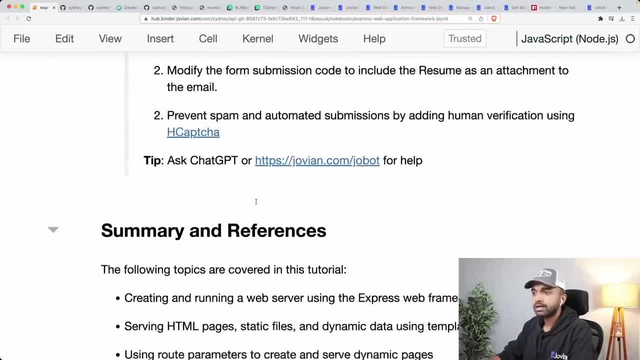 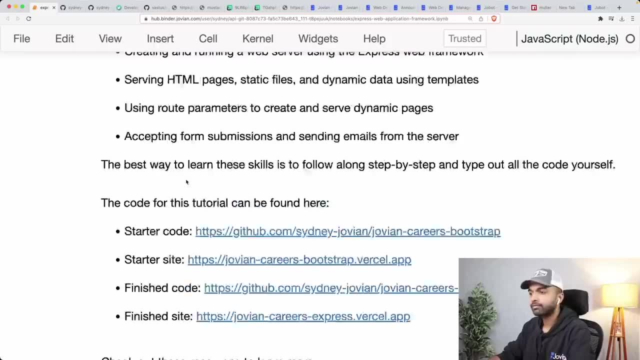 NodeMailer, SMTP, all of that, Okay. One exercise I would definitely encourage you to try is to modify the form submission code to include the resume as an attachment to the email. That'd be a very interesting thing for you to try, Okay. 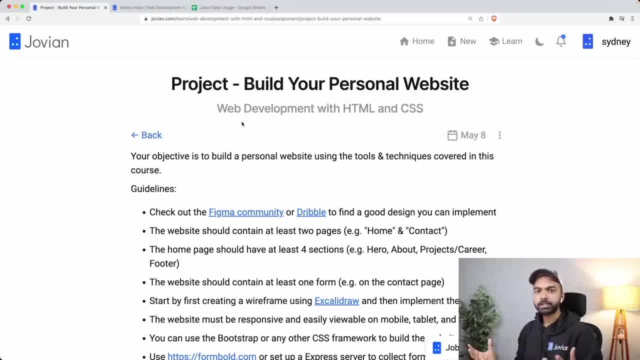 Now, your objective with this project and with this course really Is To be able to build an entire website by yourself, from scratch. So you're going to build a personal website using the tools and techniques that we've covered in this course. Okay, 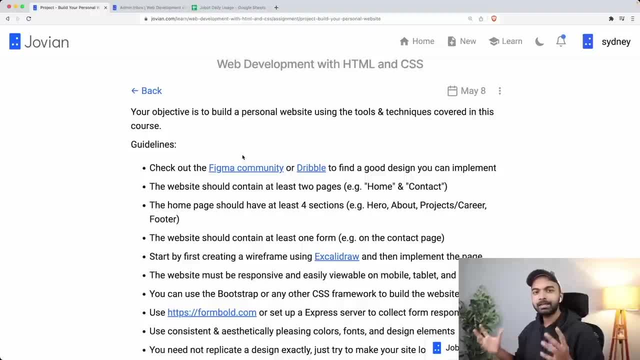 Now, of course, this is not a web design course, and design is its own entire area. that might take several years to perfect, So that is why I would not recommend trying to design a website from scratch. What you can do is Check out. 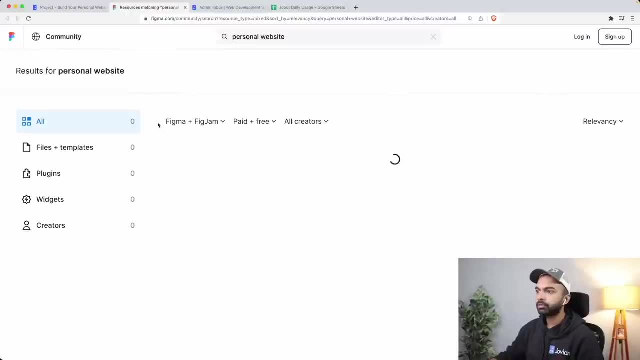 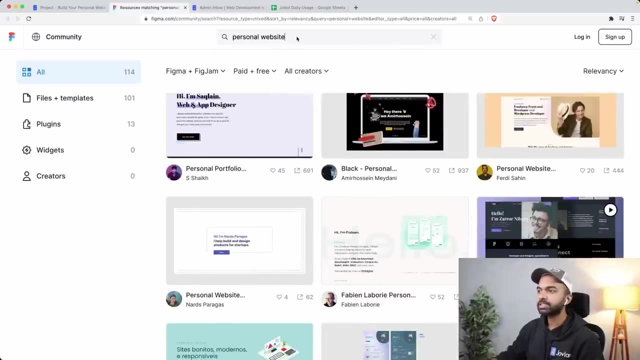 The Figma community over here. So this is the Figma community If you just go to figmacom slash community. So Figma is a design platform- web design platform and just search for personal website, You should be able to find a bunch of interesting personal website templates that you can use. 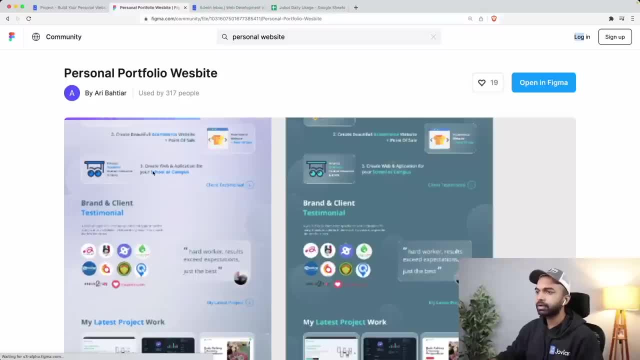 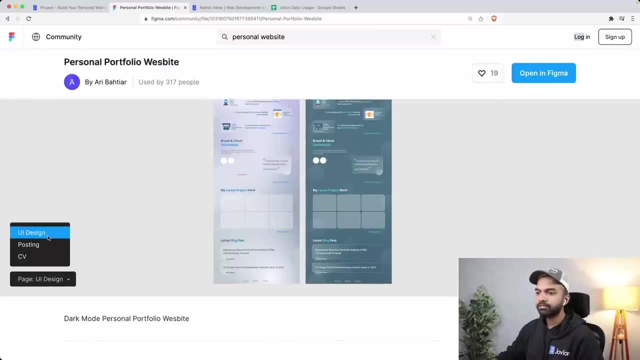 So, for instance, this one looks interesting. Let's take a look at this, And whenever you open up a Figma community project, you can actually go in and you can check out what pages they've provided. So yeah, this is a UI design. 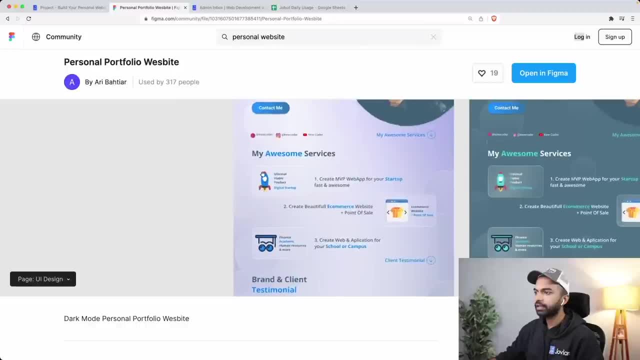 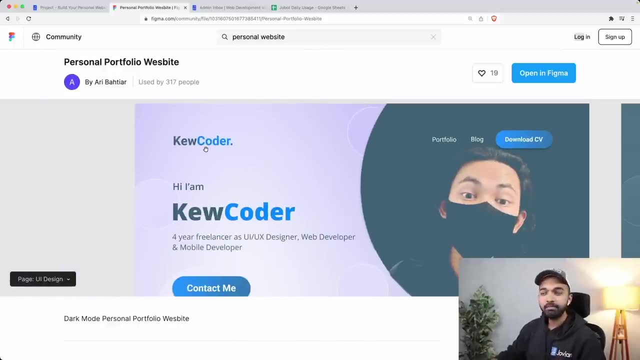 Yeah, This is a UI design page And on the UI design page you can see here that this person has created two versions that you can use either of these versions. Okay, They have a, they have a name. then they have a couple of links and a download CV button. 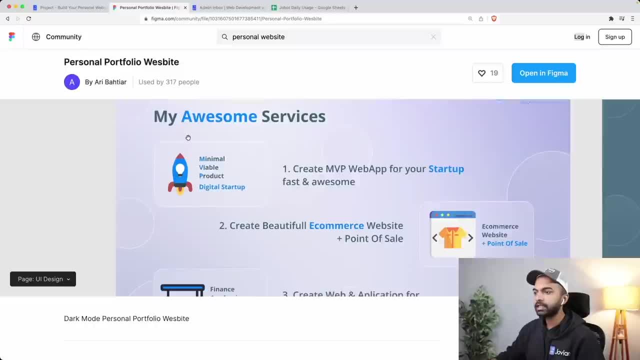 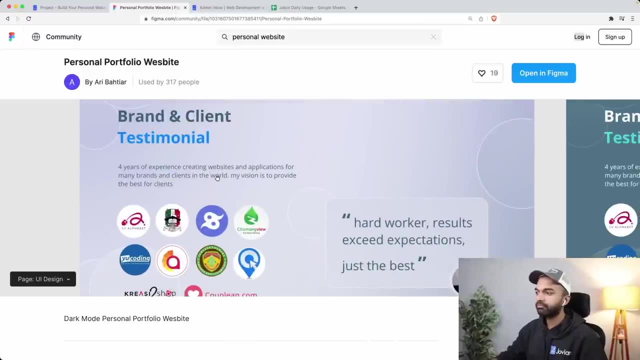 And then they have like this hero section. after that they have their social links. after that, Okay, They're talking about some of their services. This is where maybe you could talk about your education, your work experience. Then they have maybe some projects that they worked on, like this: 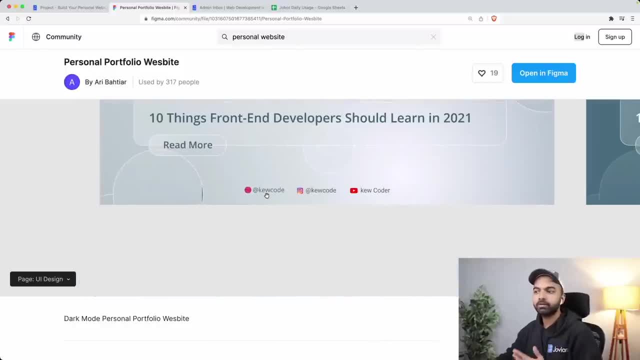 I listed here and then they have maybe some blog posts. So if you have some blog posts that you've written on medium or elsewhere, you can link those as well And they again they have a footer with some social links, right. 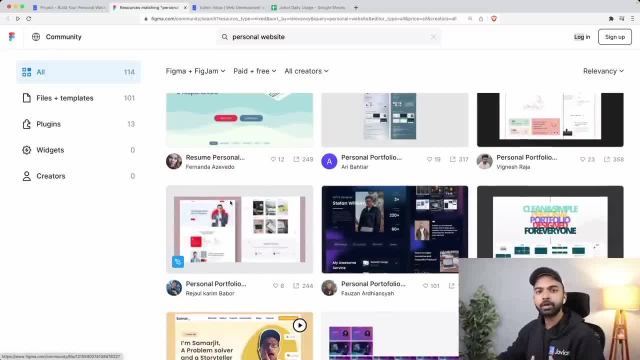 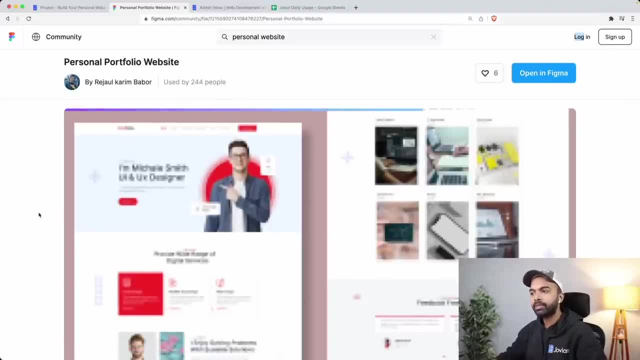 So you do not have to- and I want to stress this again- you don't have to try to design your own webpage. I would not recommend doing that, because that's not what this is about. It's about being able to code your own webpage in HTML and CSS and make it look good. make. 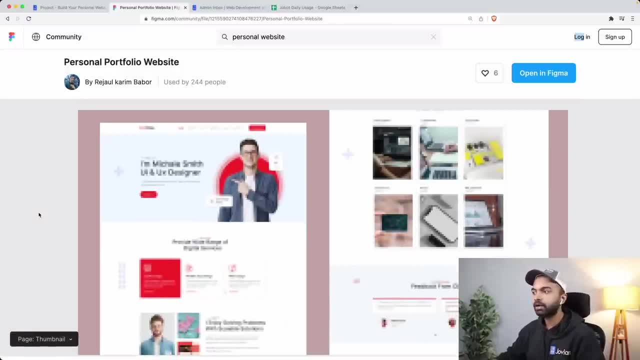 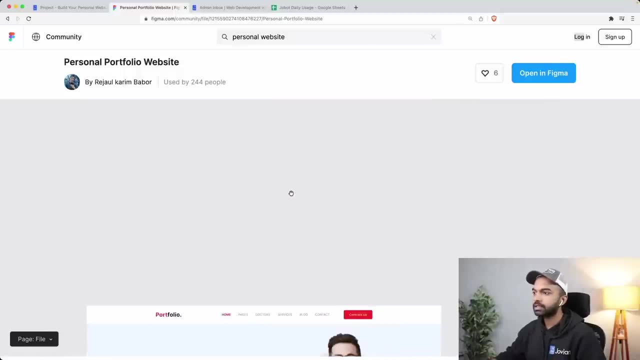 it responsive, use the tools, libraries, frameworks that we have covered in this course. Here's another example. Okay, So again, let's go into this. So here again, there seems to be this section over here, there is a nav bar and then a bunch. 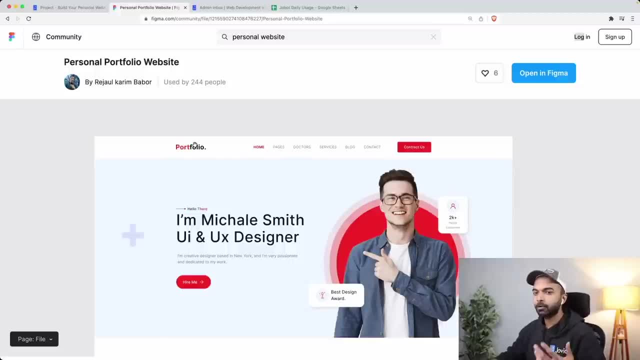 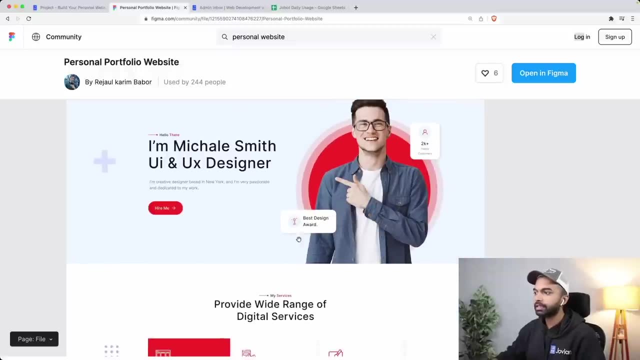 of links here, So it's not that you will use these exact same links in your project. What you're going to do is you're going to replace it with some of the links or some of the items that make sense for you, And there's a zero section. 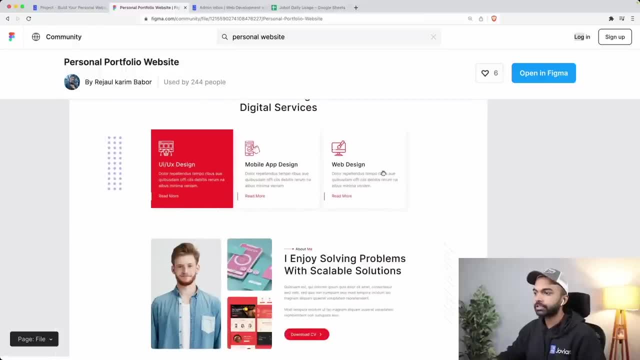 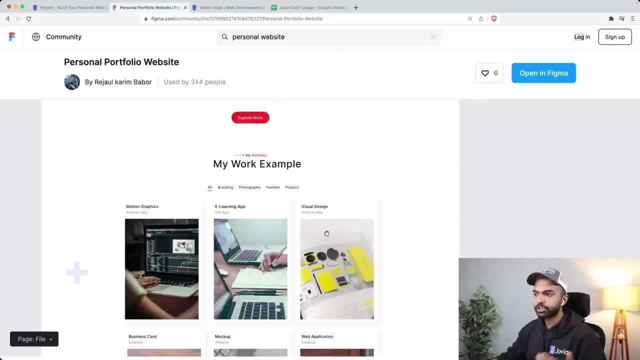 You can probably put up your own picture here. And then there is a bunch of services as an about section. There's a bunch of project sections, a bunch of cards here, And then just more things here, right? So it's again. you don't have to use all of this. 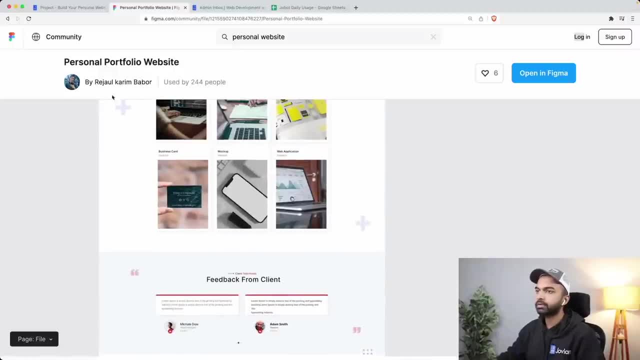 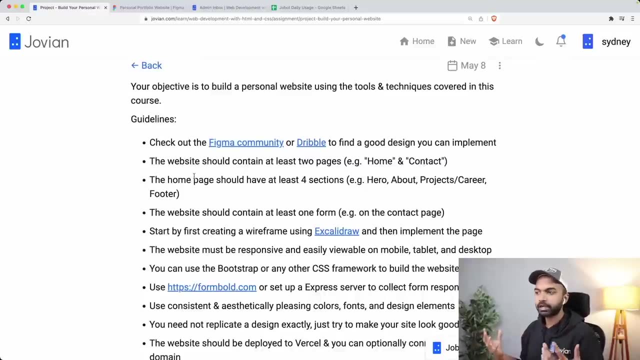 You can just use some of this. Then there's a contact form here as well, and so on. So I just want to go over some guidelines here. So there's no tutorial here as such for this, because I want you to just try and do this. 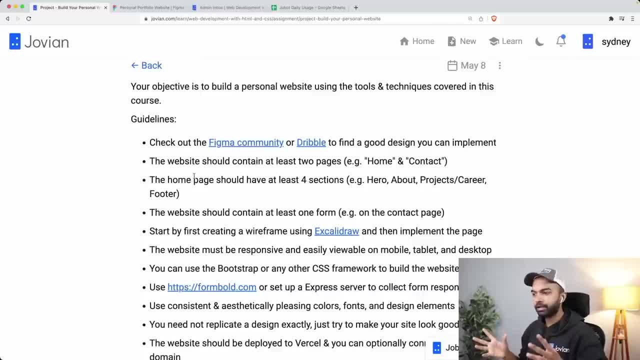 on your own. This is the first open-ended endeavor in terms of web development, So there's not a lot of step-by-step instructions. It's a bit open-ended for you to go out. check out the Figma community. check out Dribbble. 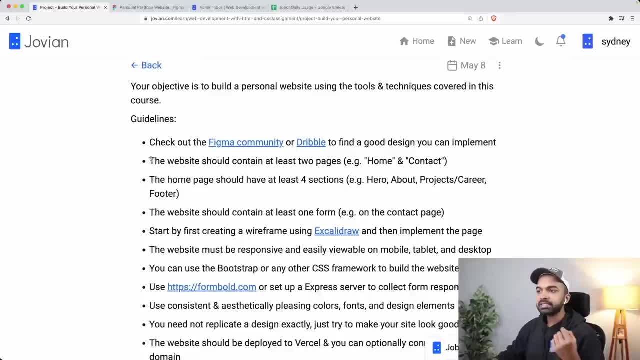 find a good design that you feel you can implement, Then here are some requirements that your website needs to satisfy. Now, of course, feel free to do as much as you want. feel free to go as deep as you want and as broad in terms of the kind of content you want to incorporate. 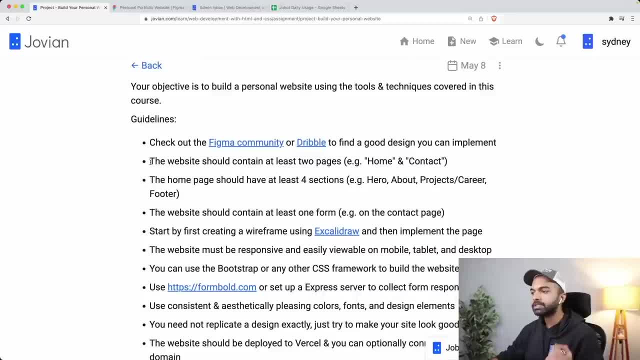 But the key things that you will need to keep in mind is this: that your website should contain at least two pages, And I would recommend these pages can be home and contact or, if you want to spread them out into multiple pages, If you want to have home as one page and then maybe projects as another page or one page. 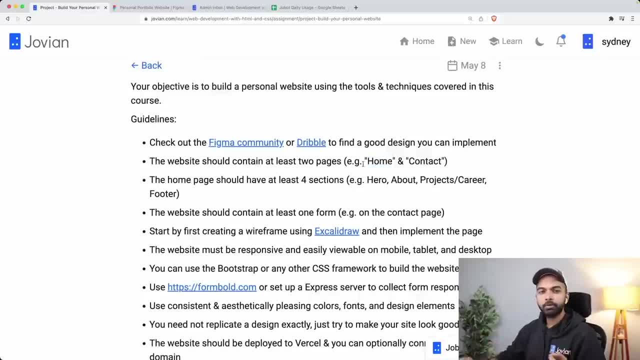 per project or something like that, You can do that as well. Or if you want to incorporate a blog of some kind into your website, you can do that as well. But for the purpose of this project, we require your website to have two pages. 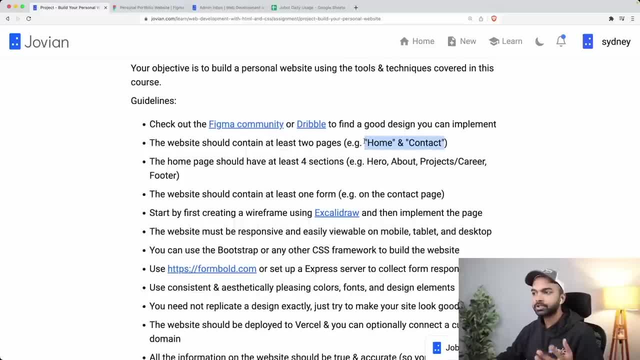 All right, Not more. you can have more than that, but at least make sure that you have to. not one will not do. second, The homepage should have at least four sections, and by section we mean so, and that excludes the navbar. So this is one section. 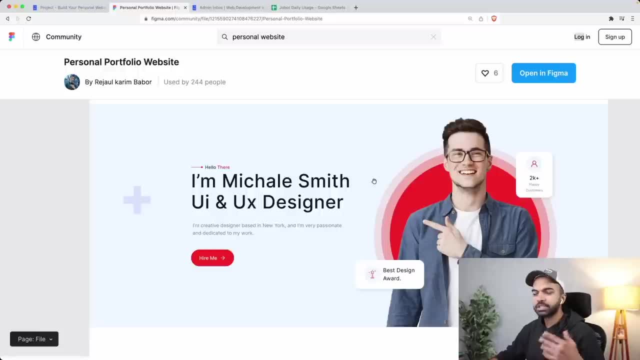 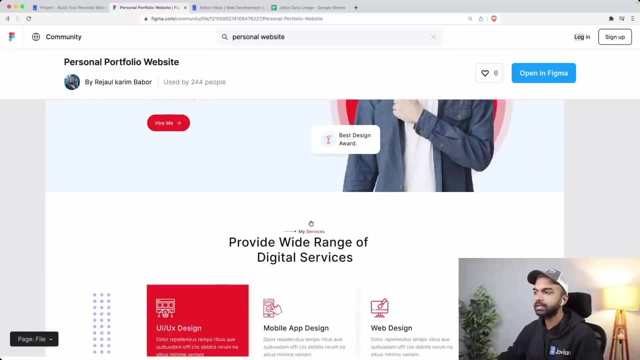 You can see here This sec. This is generally called the hero section because this is where you kind of put it and put a picture and just say some, say something with big text, So it's just welcoming people. Then you have maybe you can have maybe a work experience section. 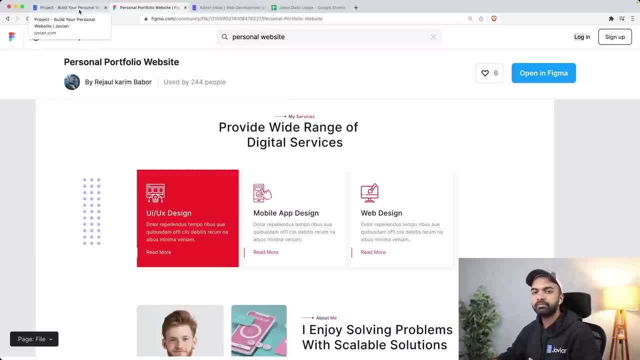 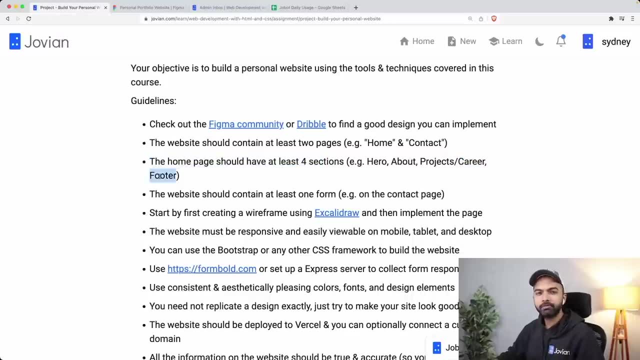 You can have maybe a project section. If you don't have a lot of projects, you can have maybe an education section or something like that, And then finally all you can just talk about your career And finally maybe you can have a footer. 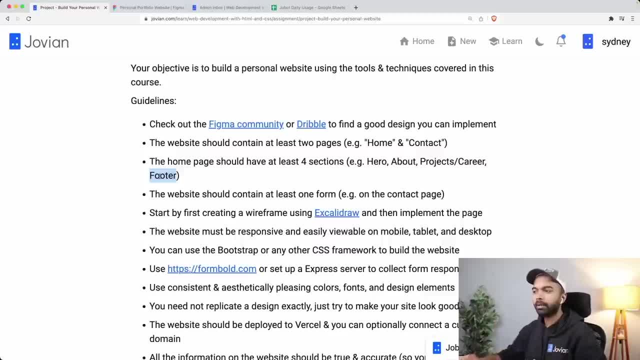 You can have, maybe just like a small note about yourself, Maybe just sharing your basic, your, your life journey so far or some just something very basic that would be informative for a potential employer. So when you go out later down in the bootcamp and you go under and apply for a full stack, 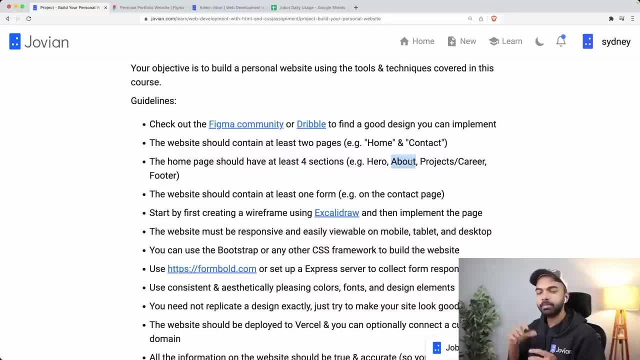 developer role and you share the link to your website. So keep in mind that. what do you want people to see when they click on the website link in your resume? Now, what is it that you want to say to them? Right, You want to present, you want to tell your story very briefly, just like you do on a 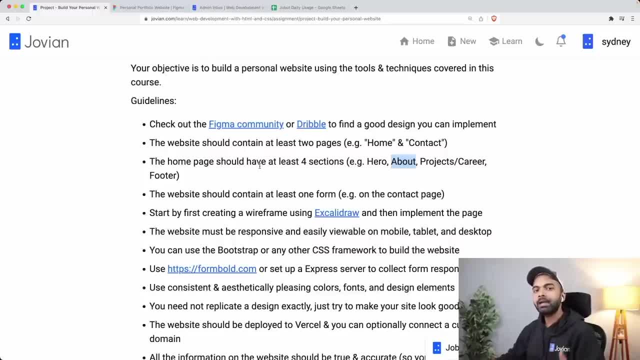 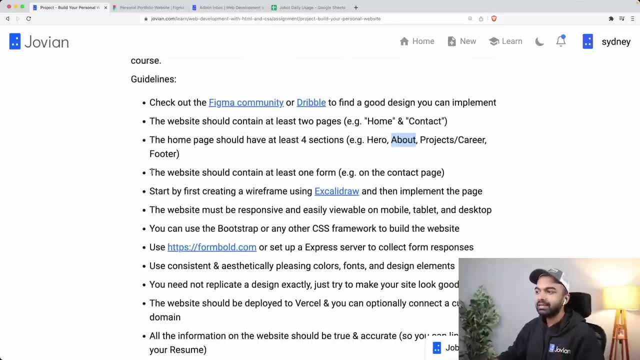 LinkedIn profile, For instance, and you want to present some interesting work and you want to showcase that you have what it takes to build good, good looking, responsive websites. Okay, Then the website should contain at least one form, And I would recommend this. 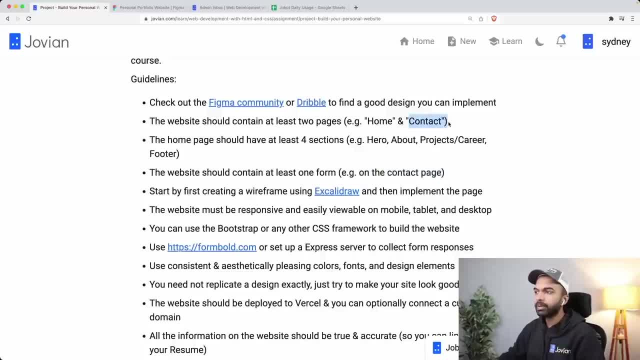 It could be a contact form, So you can. maybe if you have a contact page on the contact page you can have a contact form, or you can have a if you're. if you don't have a contact page, you have a different. 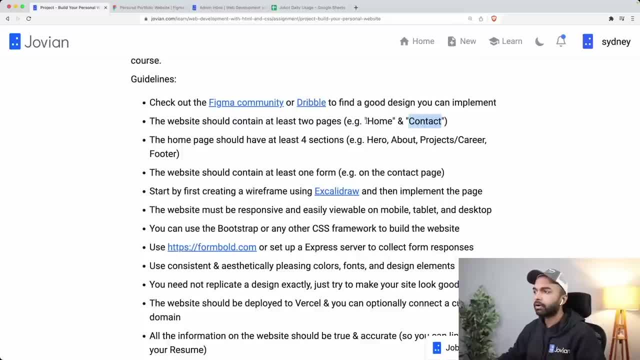 page for something else, Then you can maybe just create a form for on the homepage itself, but make sure that it has at least one form that maybe at least three or four fields. typically they would be email name or your, your message or something like that. 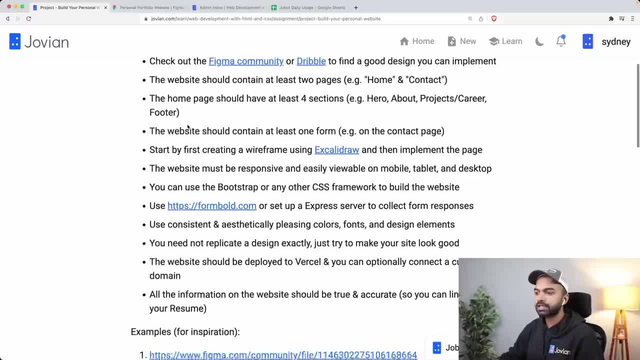 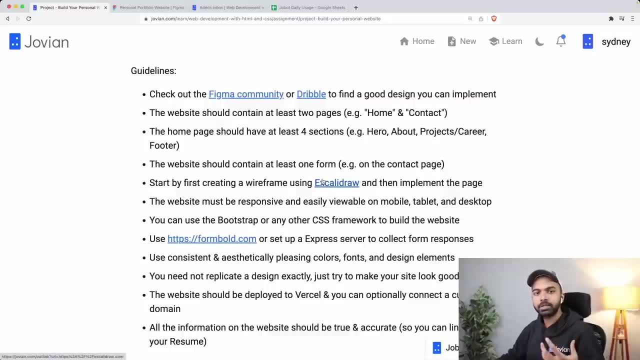 And I would recommend that, as you browse a few of these examples- and we have included several examples here- start by first creating an, a wire frame, because that is what we have been doing so far. Right, So follow that procedure of creating a wireframe, even if you've picked a design because you're. 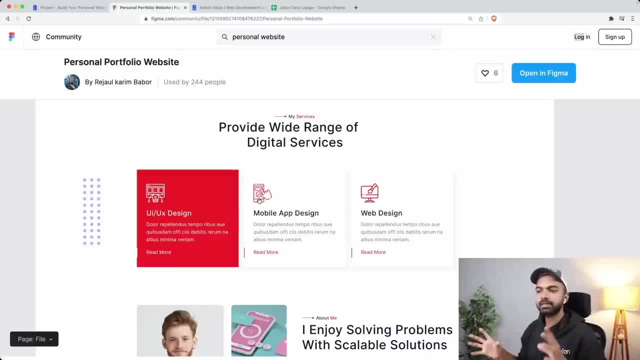 not going to implement a design, exactly like you are going to change the design or you're going to Create a content that is going to make more sense for you or your website. So start by just after having selected some design or after having just figured out what. 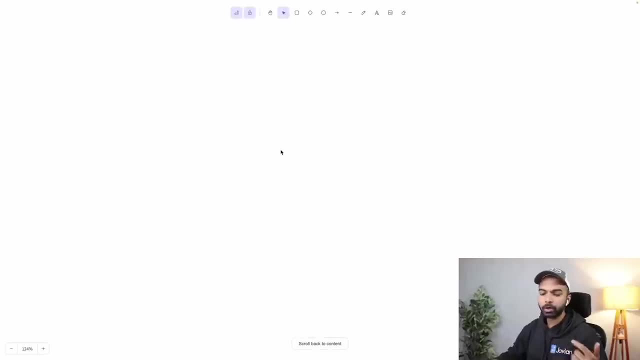 you want to show. start by first creating a wireframe so that you can figure out what content you want to put on the page Right. So, for instances, if I were creating my personal website- my personal website- I would maybe- let's see. 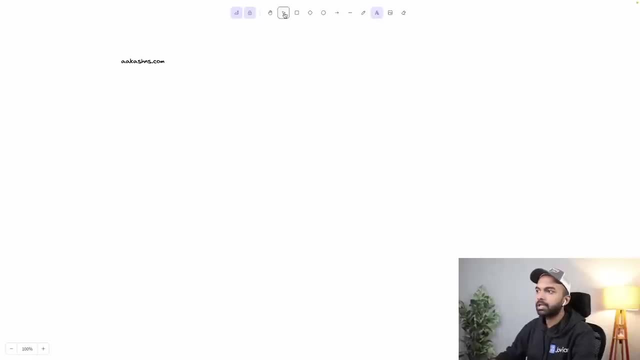 So let's say I were creating our passion: iscom. That is my, that would be. I would probably get that domain. That is my personal website. and here, what would I like to put? So well, I would like to definitely have a navbar at the top and in the navbar I would. 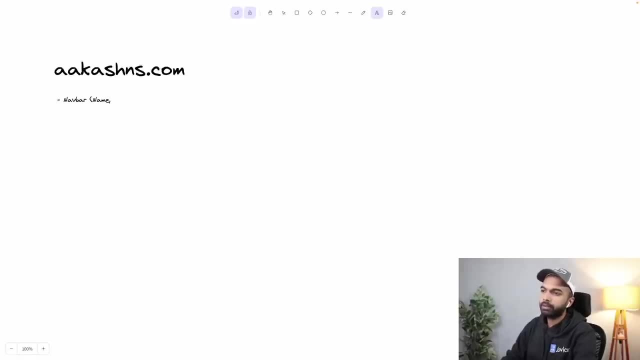 want to mention my name. I would want to mention maybe like the home link and maybe, let's see, I would like to mention a contact page link, something like that. Right, And then, all after the navbar, I would want to have maybe a quick hero section. 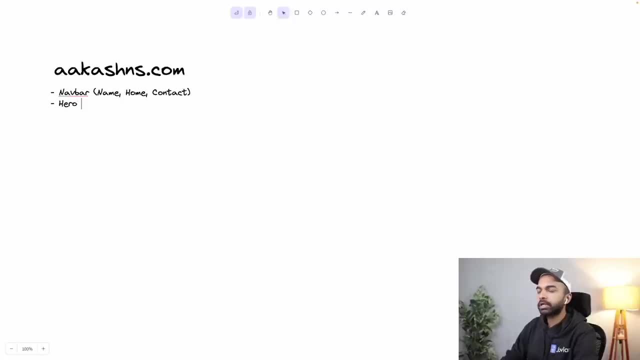 Let me just put in that information Here and then we'll draw the wireframe, a hero section, And in the hero section I will probably have maybe a photo, maybe a heading like a big title: hi, I'm Akash, or something like that. 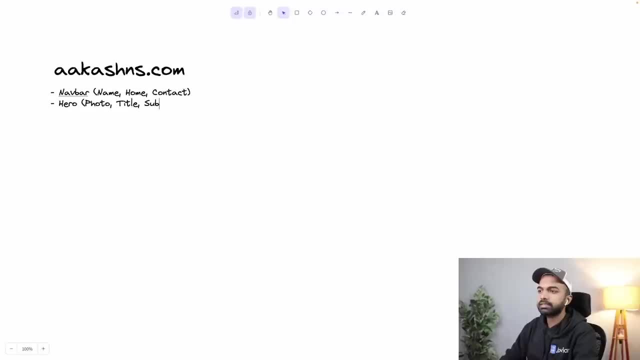 And maybe a subtitle- Let me just call it title and subtitle, right, Something like that. So that would be the hero section. Then maybe I would have an about section. in the about section I would create a short bio, something like: Hey, I'm Akash, I'm from such, I'm from India. 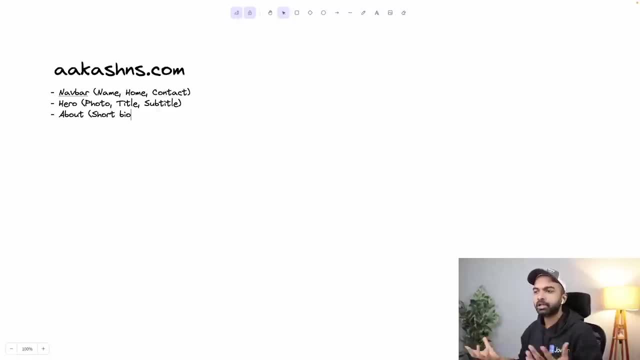 I live in Bangalore, I do this, I do that, I've done this in the past, etc. Thanks for checking out my website. feel free to contact me, right, something like that. So that would be good. Then I would probably want to include maybe my projects, because I think that would be. 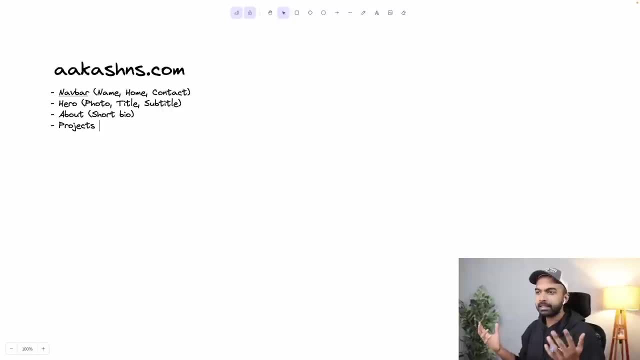 the most interesting thing that I would want to showcase, all the interesting things that I've worked on over the years. So I have a bunch of like Android apps, websites, courses, etc. I would mention those then maybe I would want to- let's see, I would want to maybe talk a little bit about my career. 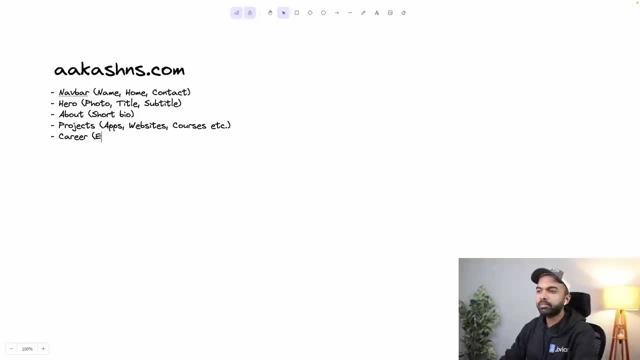 Right. So in this I would probably mention my education, And I would probably combine education and work experience, because I've just had one job, full time job, And after that I've just worked as a consultant and so on. So yeah, education, work experience, etc. 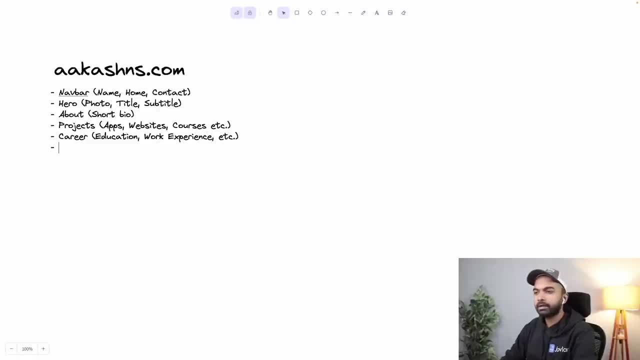 So I will do that. then I would probably just have a footer, And here I would put some social links. And then I would probably just have a footer And here I would put some social links. I don't have social links, but I would probably put like some external links. 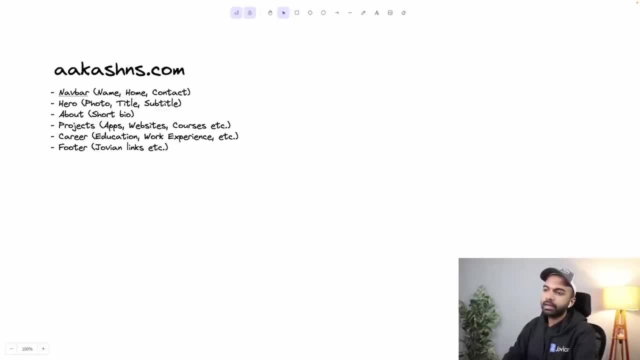 So like Jovian, Jovian links, etc. Right, And maybe I might also have one section here where I might highlight some of my best work in terms of videos, So like we had some YouTube videos like that, Alright, so that would be what I would want to put. 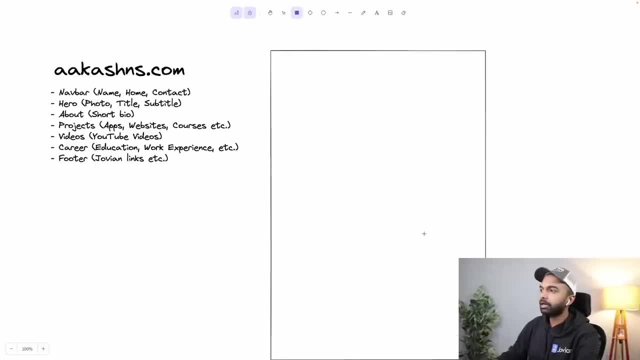 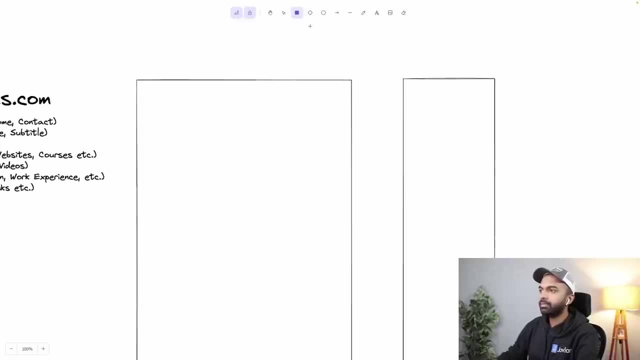 So then what I would do is I would try to create two wireframes. I would try to create one wireframe for mobile And one wire, one wireframe for desktop. So I would just put it like that, maybe, and I would say: okay, this is my desktop wireframe. 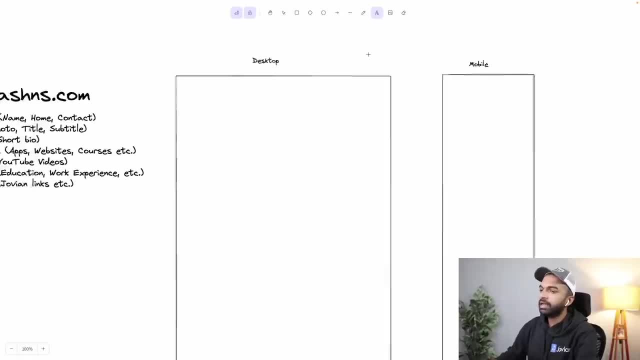 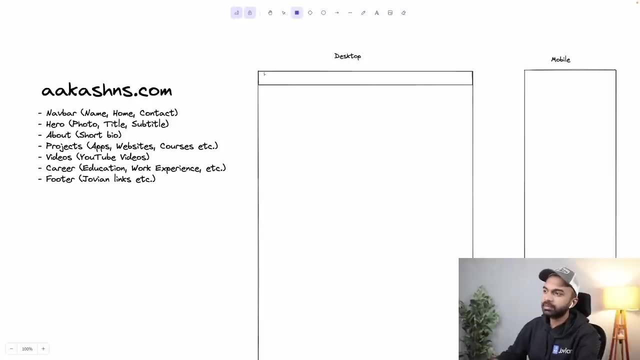 And this is my mobile wireframe, Alright, and then, as you can imagine, I'm basically going to just put a bunch of boxes here, Okay, so this is going to be my navbar and I can just fill in some information into my navbar. 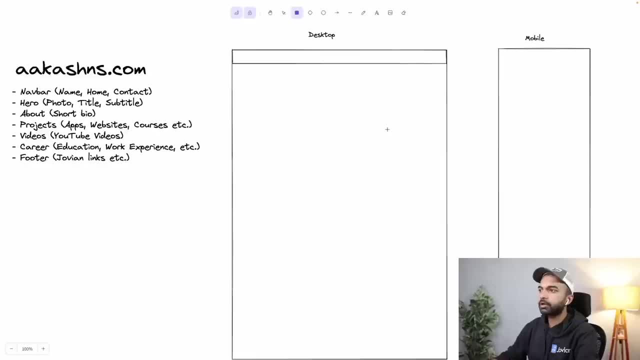 And again, you can do this on paper. I'm just showing this to you here on this tool, Excalidrawcom, but you can do this on paper. So that would be the navbar, and then I would have a hero section here. So I would kind of leave some space for the hero section. here is where I would put the 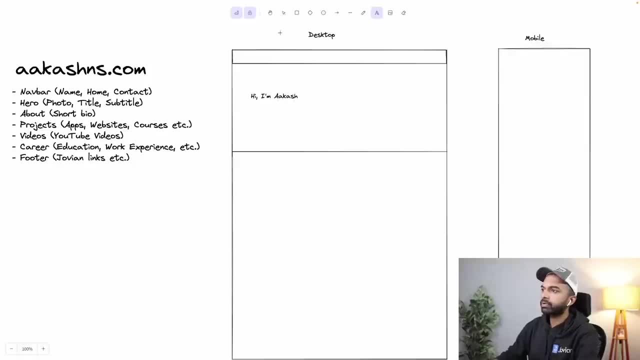 title something like: Hi, I'm Akash, like that, And often when I'm doing this I would even just pre draw, So I would maybe just do something like that that. okay, maybe here I want to put like a picture of myself saying hi or something, and maybe have like a couple of lines of introductions. 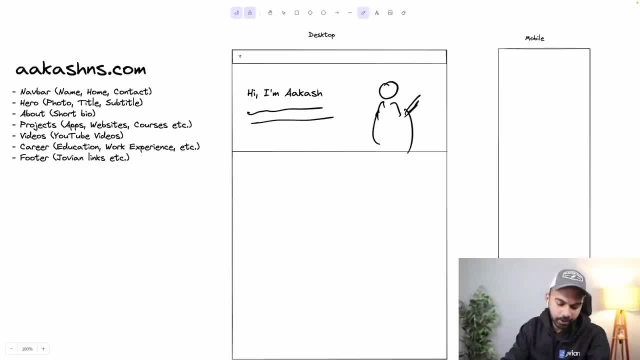 Okay, Okay. So here I have the introduction about myself. here I might want to again mention my name. here I want to say home contact, something like that. then I have the about section, So that would be something like about me, and then I would have maybe a few few lines. 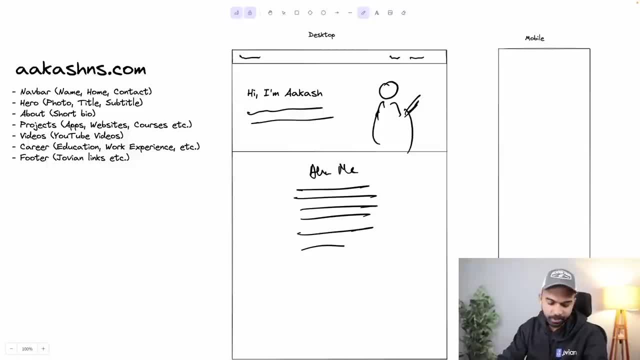 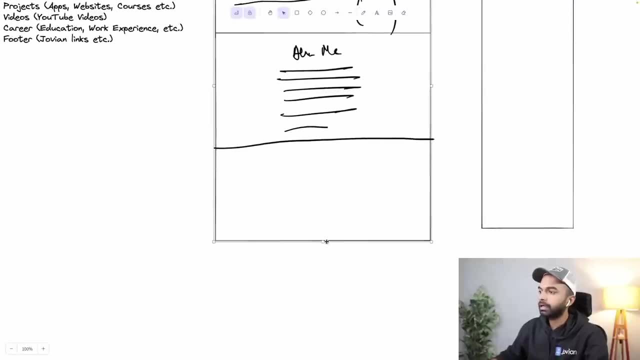 of text about myself. I could also maybe put a picture on the side, but I think that's fine. So then, after the about section, I would probably then go down and then create a project section, And that's where it's a good opportunity to create, use some cards, maybe. 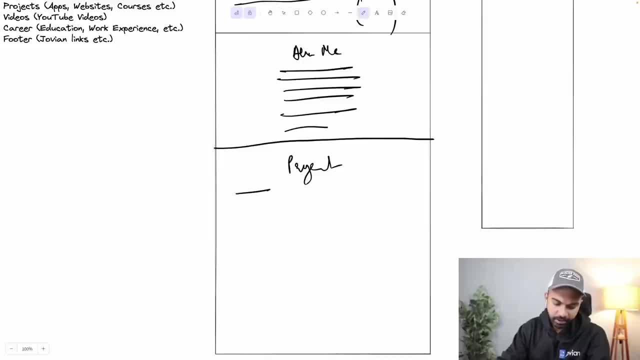 So let's see Projects, and I would probably just put a bunch of cards here like that, maybe three cards or so, And then I would maybe just put a button saying view more and maybe there could be a separate projects page that goes in there. 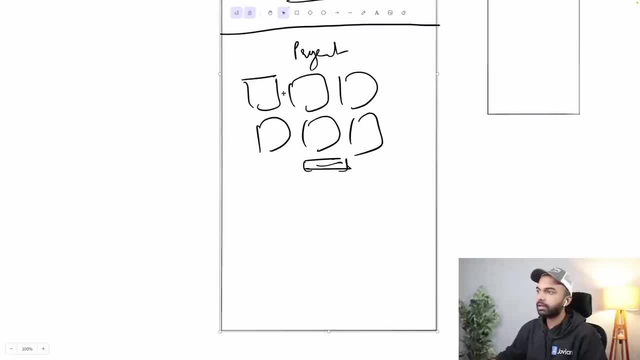 And, yeah, feel free to get as detailed or as rough as you need, But the idea is, you want to lay out all the content that you want to add here So that when you are actually implementing, you don't really have to think about what. 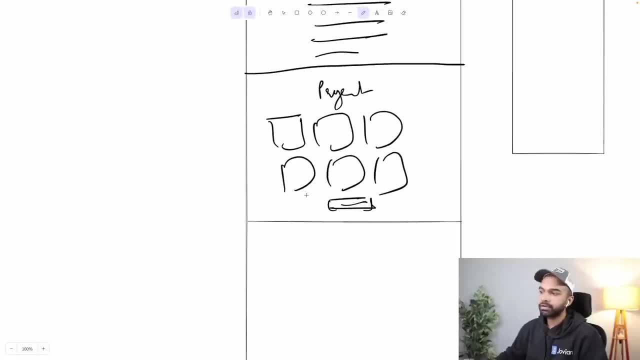 content do I want to put here? right? Then, okay, we have videos, So I would probably put a video. Okay, So I would probably put in some videos here. So let's see videos Again, I would probably just embed a couple of YouTube videos here, like that. 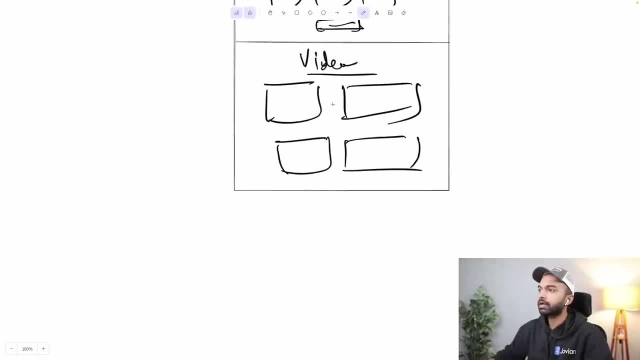 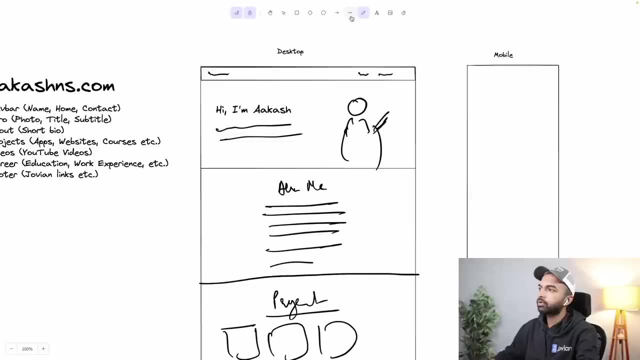 And maybe have a line describing what projects, what, what videos I've done and so on, And then I would adapt it to the mobile view. So in the mobile view, of course, you would have a slightly different structure. maybe you would know you would need like a menu over here instead of an actual buttons. 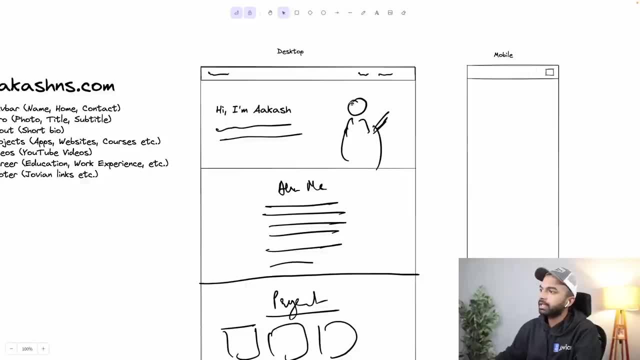 So I would probably have that menu button over here. I would probably take this: Hello, you might also want to take a picture, a new picture for your personal website. it would be nice. but I would probably take this like Hello thing And I'd probably just put that here. 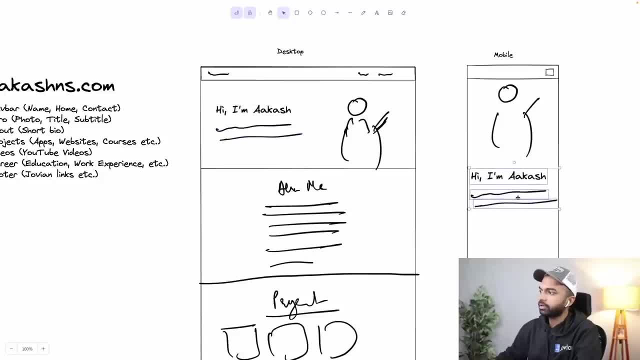 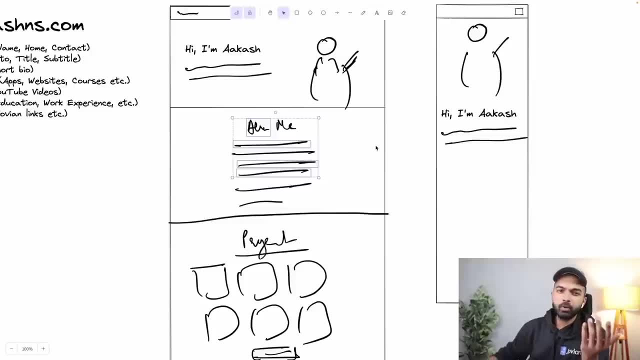 And then the hero text would probably become centered and that would come here like that, And then I would have the about me section. I think this would remain as is. So you get the idea that you want to have one breakpoint for mobile. you want to have 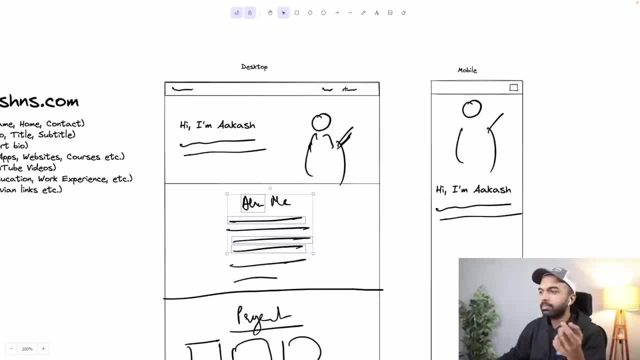 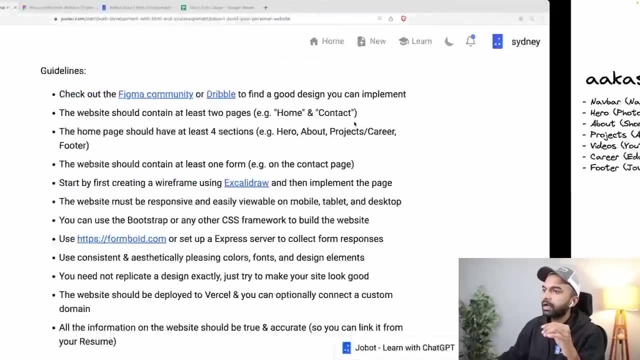 one breakpoint for tablet and one for desktop. But if you want, you can just do mobile and desktop wireframing And you, you will kind of know that. okay, this I'm going to get from this search to the styles I'm going to get from here. 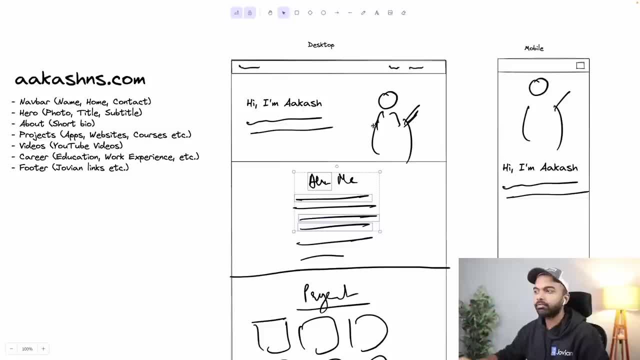 But the content and what I'm going to write here, all of that you can actually put into your wireframe. I'm not putting it right now because it'll take a while, But you can actually put all this into your wireframe or maybe into a Google Doc or something. 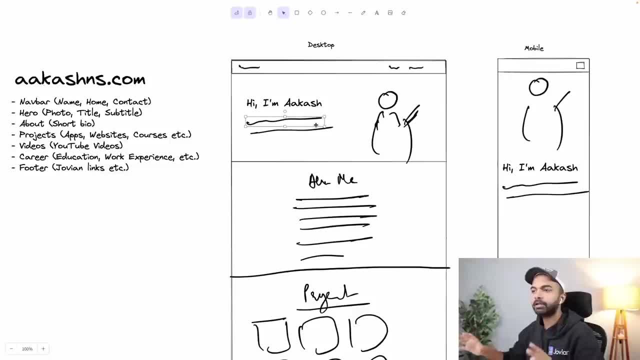 But the idea is before you even start writing your first line of HTML. You can actually put all this into your wireframe or maybe into a Google Doc or something, But the idea is before you even start writing your first line of HTML. So you are in a position where you already know what's the what the page is going to. 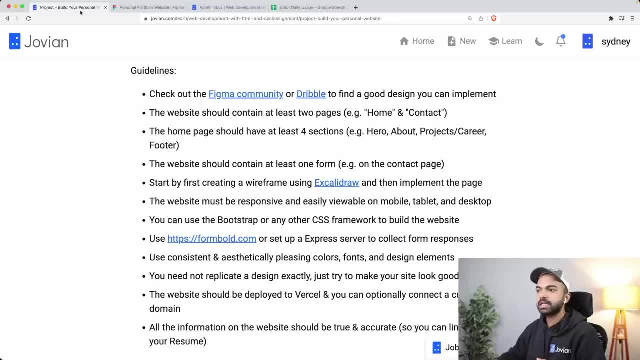 look like The biggest mistake that you're going to make- and I repeat this again- is that you start coding right away And then you're thinking, okay, what should I put in this section? And then you, as you're trying to put something into the section, you realize, okay, now the 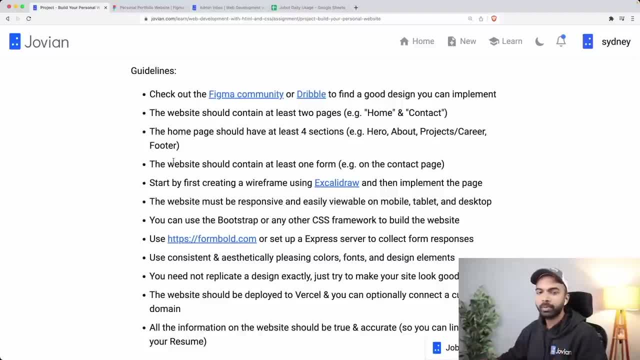 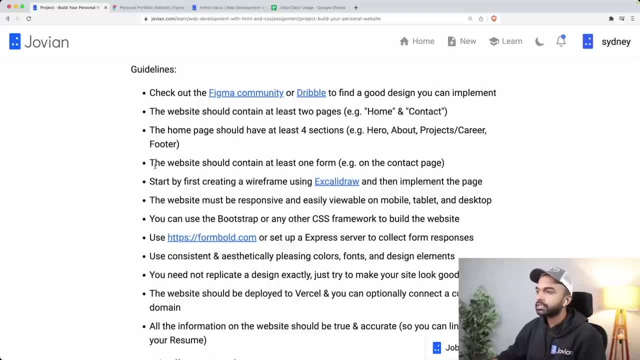 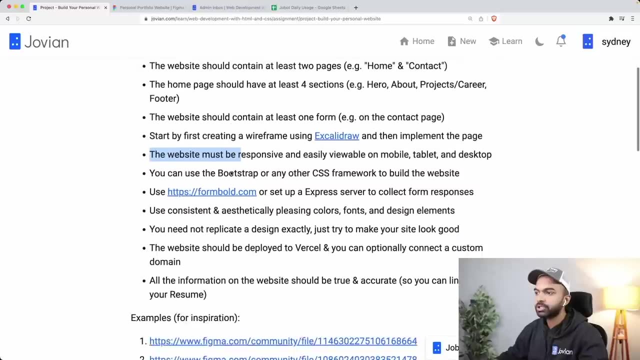 design is no longer working, or now I'm not able to make it responsive. So separate the design, content and implementation. Okay Yeah, So Once you've created a wireframe, then create once you've picked a design for inspiration. 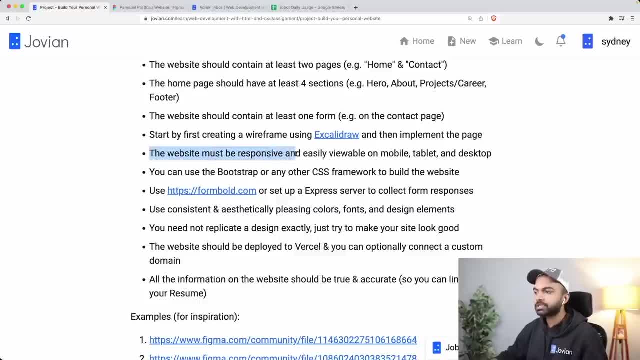 then create it section by section, and the website must be responsive and it should be easily viewable on mobile, on tablet and on desktop. Okay, So make sure to test it on real devices and make sure, of course, you can deploy it to. 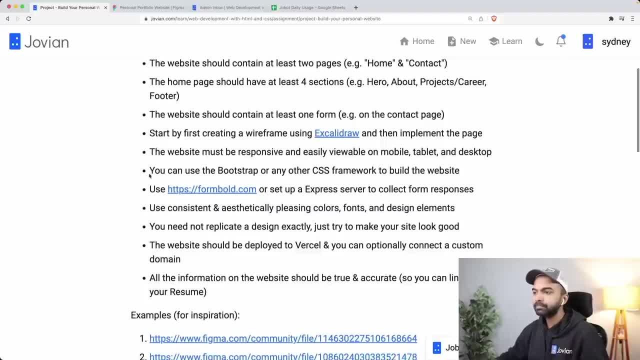 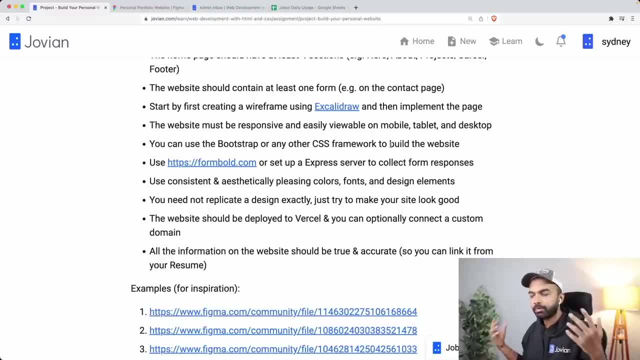 Vercel. You can open it up. You can send yourself a link and test it Now. you can use Bootstrap or you can use any other CSS framework. you want to build a website. If you want, you can do it without Bootstrap. 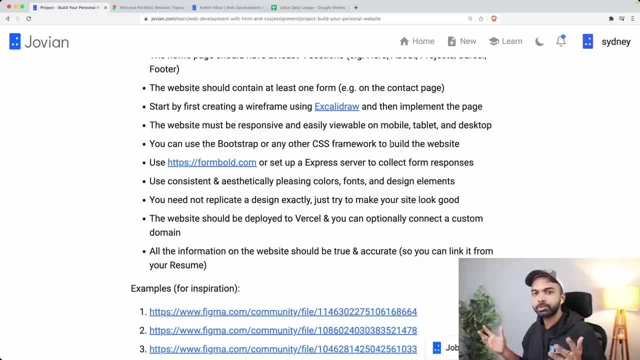 Feel free. This is an open-ended project. We are not forcing you to use Bootstrap. You don't have to. but if you want, you can use Bootstrap, That's fine. Or you want to use some other CSS framework, That's perfectly fine too. 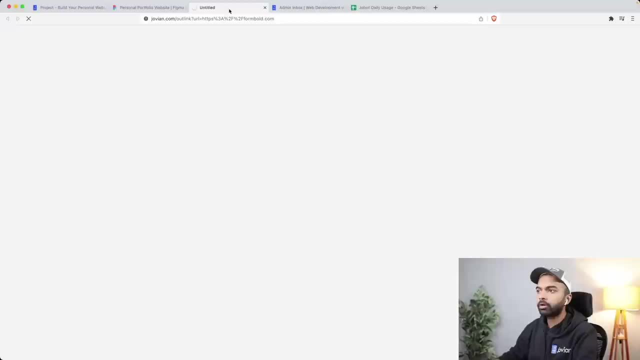 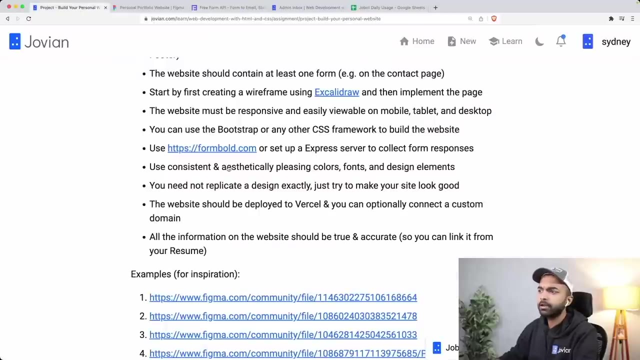 Now for the form that you create. you can either use formboldcom to collect the responses using- and we've covered this in one of the lessons, probably, I believe, the second lesson- or you can set up an express server, an express web server to 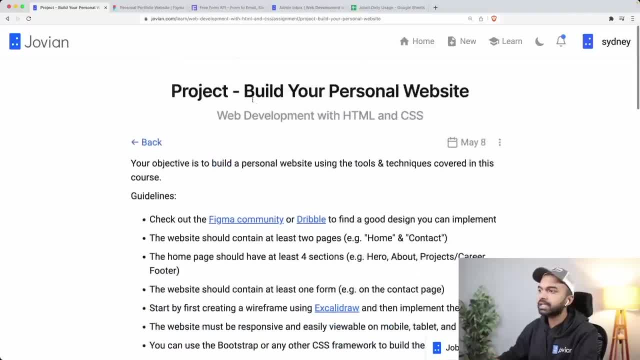 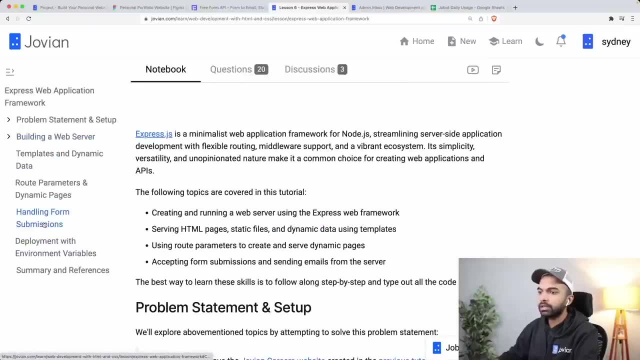 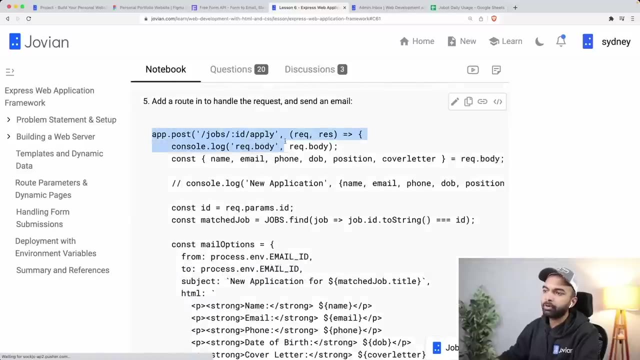 collect the responses. So again, this is covered in the previous lesson. So in the lesson express web application framework. you can see here that we have a section on handling form responses where we basically used- we created an apppost link So you can do that as well. 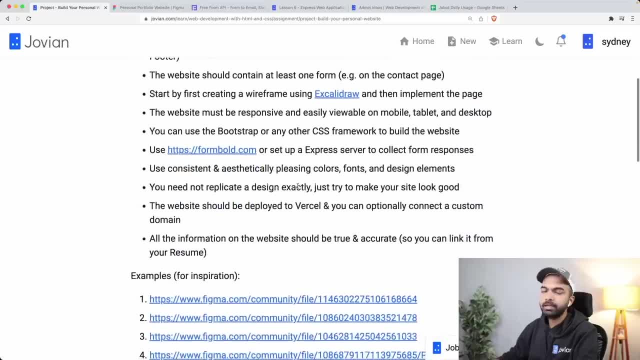 Both of these can be deployed to Vercel equally easily, So that's fine. You don't have to use express for this. You can do a simple HTML and CSS if you want. That's perfectly fine. But yeah, As a challenge, I would encourage you to maybe try try out using express. that will also. 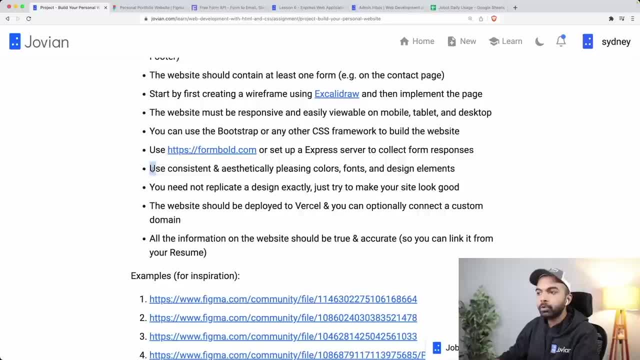 help you practice templates and other things, Then use consistent and aesthetically pleasing colors, fonts and design elements. So one of the things- even though we are not focusing on web design too much in this course- one of the things we've tried to do is make sure that our websites that we build don't 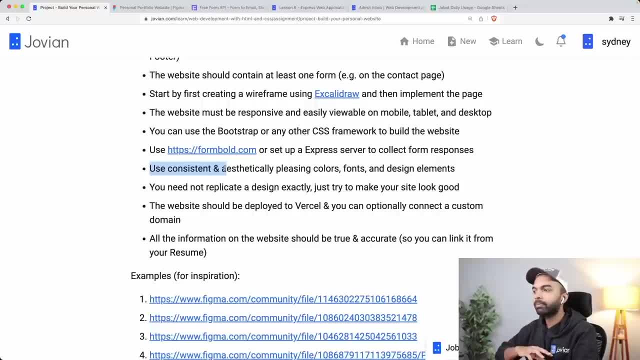 look ugly, which means that they don't have a very poor or not poor exactly, but they do not have a very well, they don't have a thoughtless or a random choice of colors, right? The default colors that CSS gives you are not great. 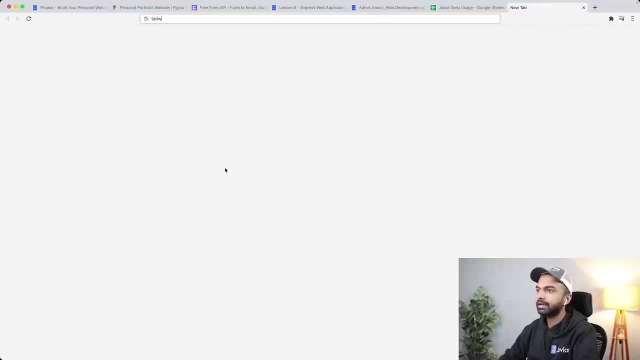 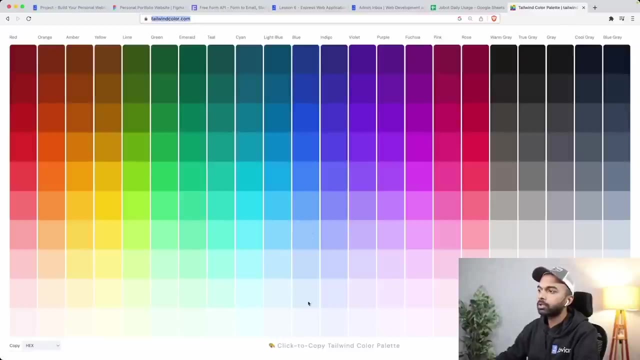 Ideally want to use a color palette, And that's where we have looked at things like tailwind, tailwind colors. It's a good place for you to pick out a tailwind colorcom. So you, you want to use a color palette. 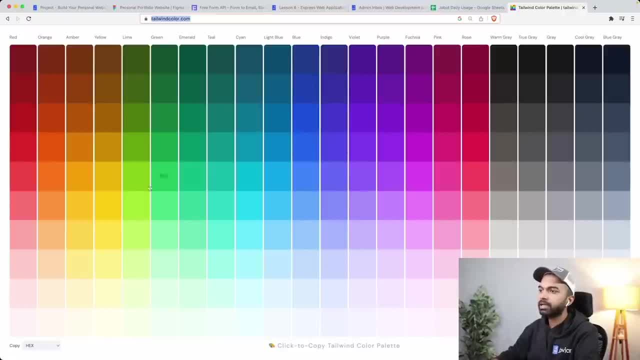 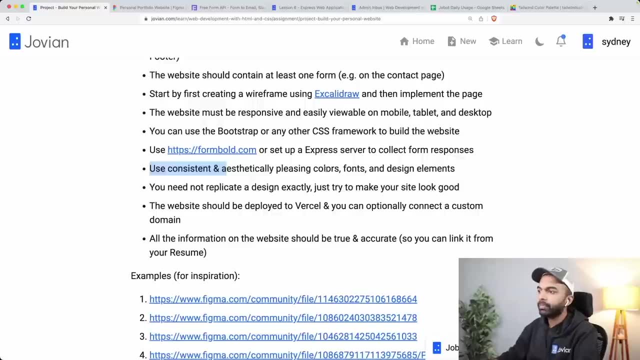 You want to have one primary color and you want to use different shades of that primary color. If blue is not your thing, pick green or pick rows or pick red, But definitely stick to a color palette and similarly fonts as well. You want to be consistent with fonts. 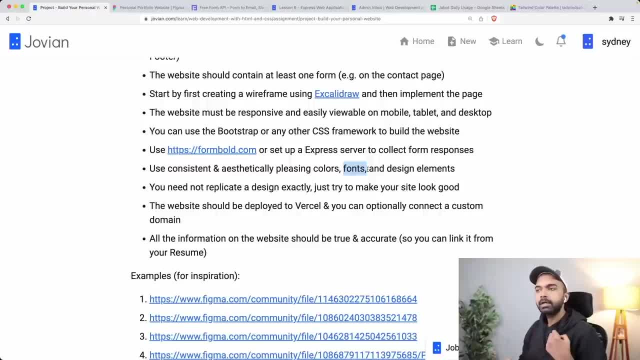 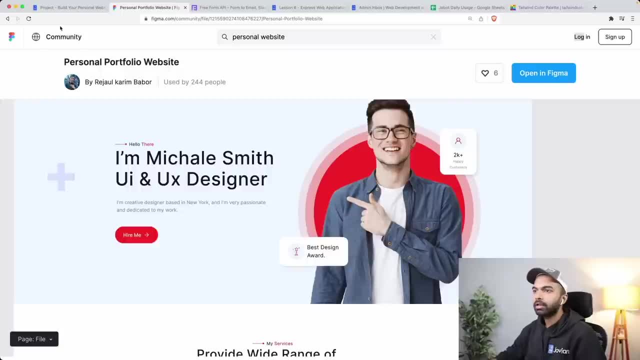 Feel free to experiment here, Feel free to try different fonts, but ideally stick to one font for headings and one font for body. Now that doesn't mean that it has to be internet Roboto Like. if I go back here on the Figma community you can see that here there's an interesting 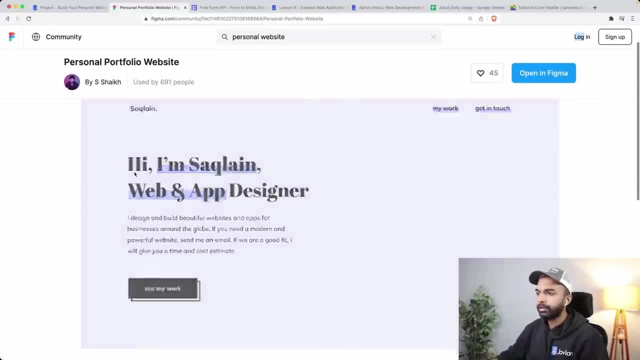 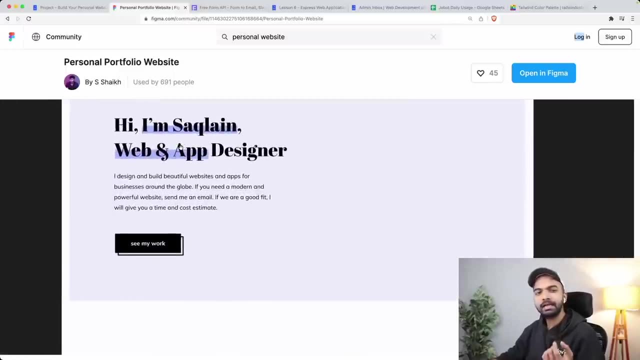 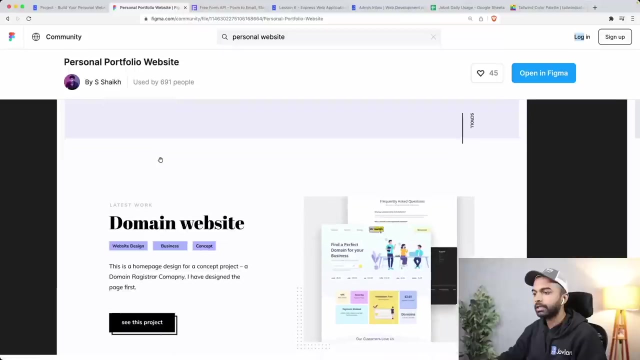 font that is used for the uh, for the header here, And that's what's called a Serif font. And in fact it's not just that: it has slight, slight calligraphic elements as well, Whereas there is a different set of uh, the different font that is actually used for the body text. 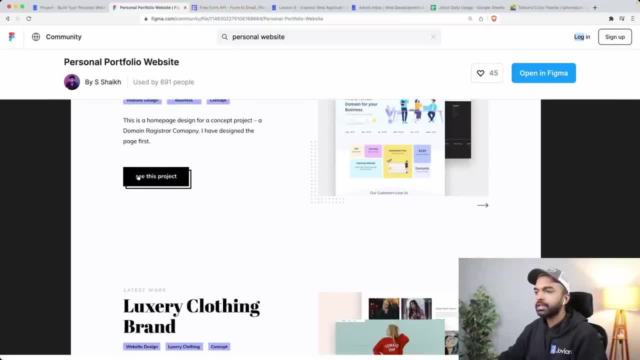 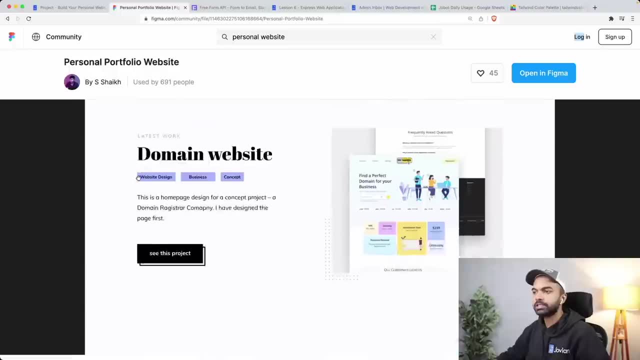 All right, And then there's this uppercase font that is used here as well. So feel free to experiment. You can use two, maybe three fonts, but make sure that it stays consistent across the page. It shouldn't be the case where you use a certain font in the nav bar. 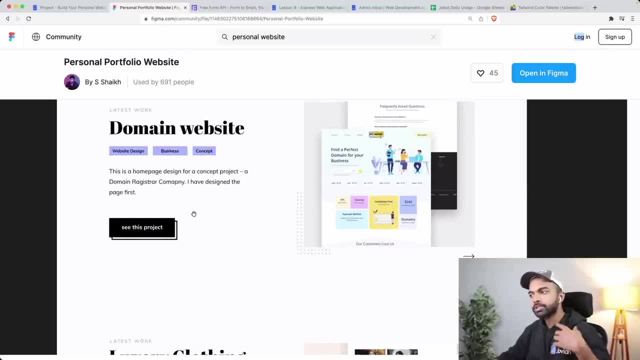 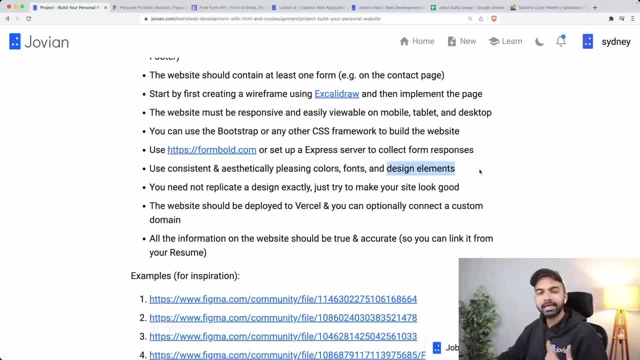 Then you use a certain font in the header or the hero section, Then you use a certain font in the about section. Please don't do that. Please keep it consistent. I hope you've picked that up, And similarly with design elements as well. 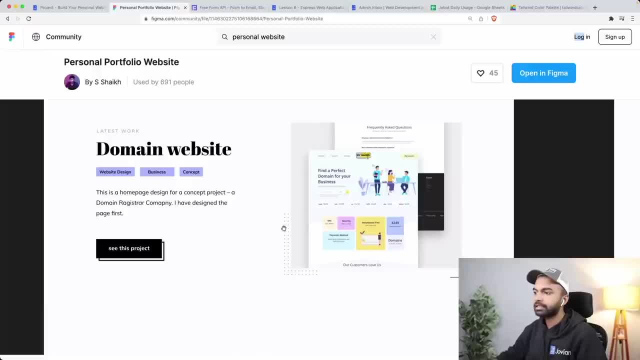 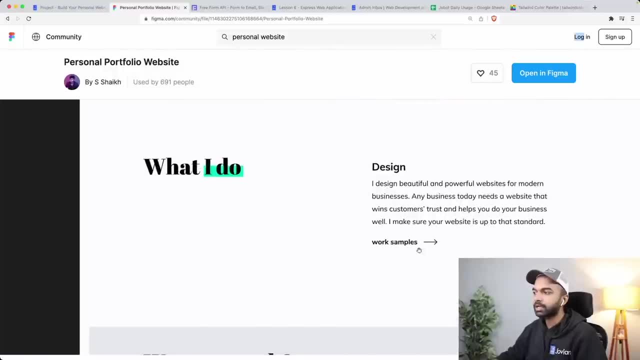 Like, if you want to spray in design elements here and there- for example, here there are these dots that are there- Um, you'll have to figure out how to actually add these design elements, but for all these design elements, keep them consistent. 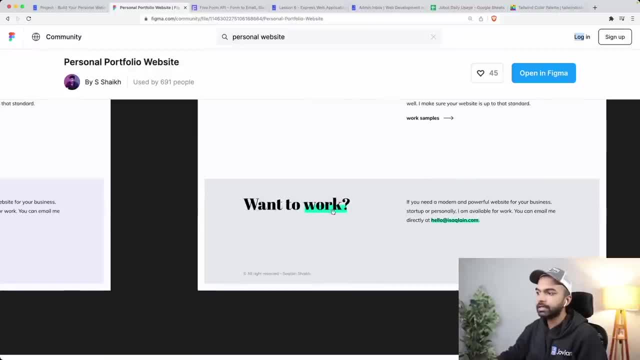 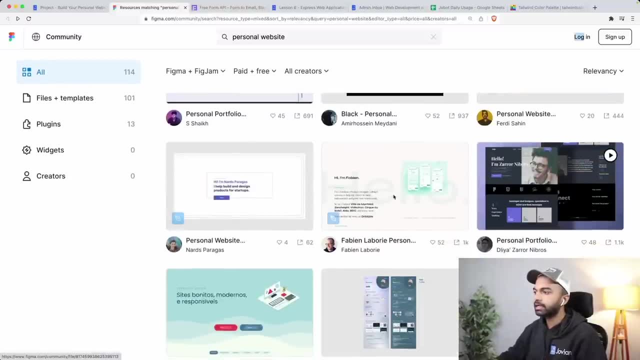 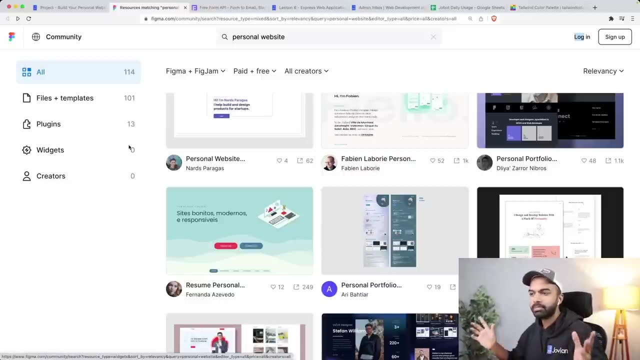 Like this arrow. you see here that arrows there everywhere. or you see this highlight here, that highlight is there everywhere as well. So, um, yeah, make sure that you are staying consistent In all of these in terms of the design. that is the key. even if it is a very simple black and white kind of page, when, when, maybe just one color here and there, consistency is key. 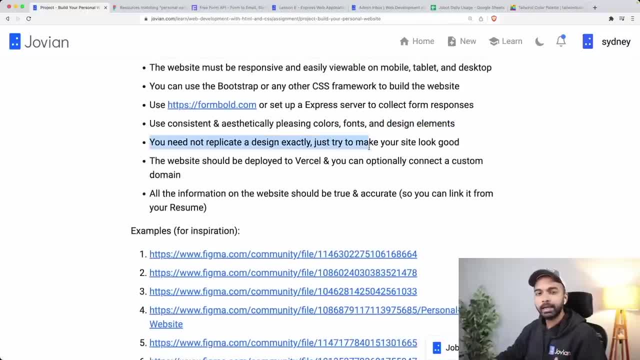 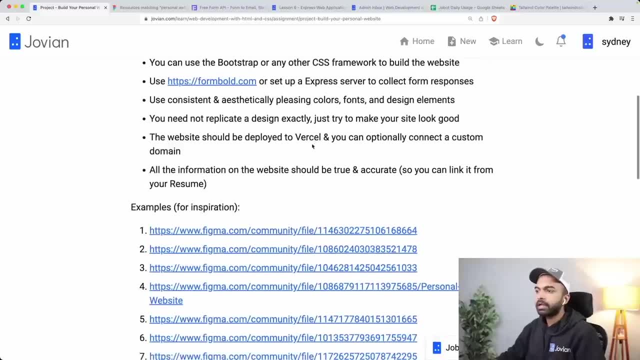 So make sure of that Now. you need not replicate a design Exactly. Just try to make your site look good, Just try to make it look consistent, Just try to make it look well spaced out And finally, your website should be deployed to Vercel. 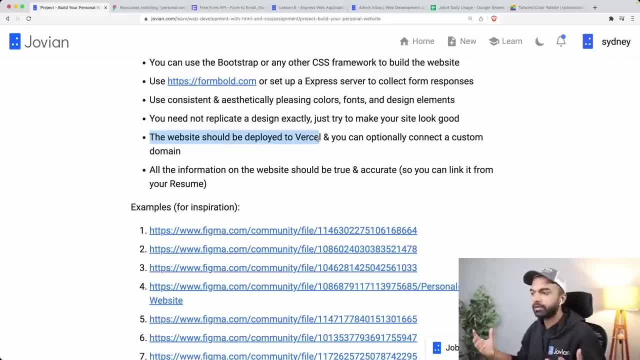 And again, there are no instructions here. by this time you should be familiar with the deployment process. So you should have to create a GitHub Repository, keep it open source, keep it public And um, then you deploy it to Vercel and optionally, if you want, you can also connect a custom domain to it. 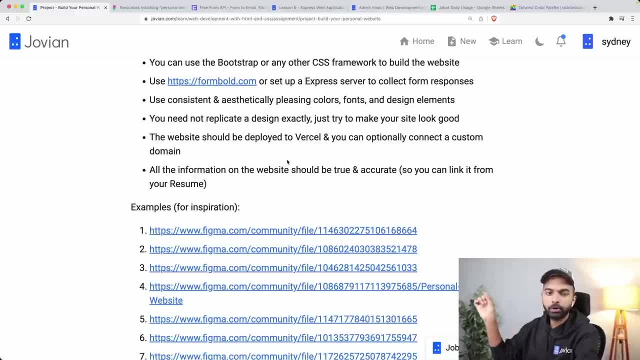 So you can go ahead and actually uh on Vercelcom. if you're going to domain settings, I let you figure it out. but you're going to domain settings and you can add a custom domain. So you can purchase a domain. 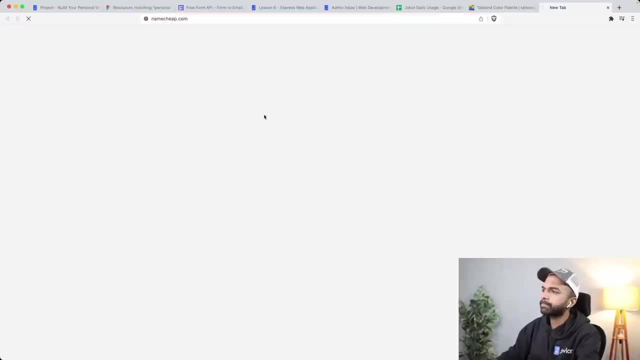 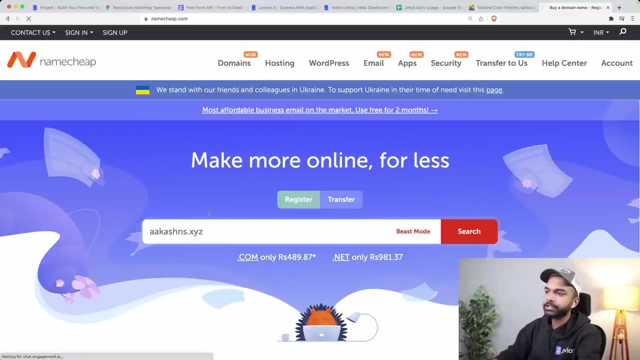 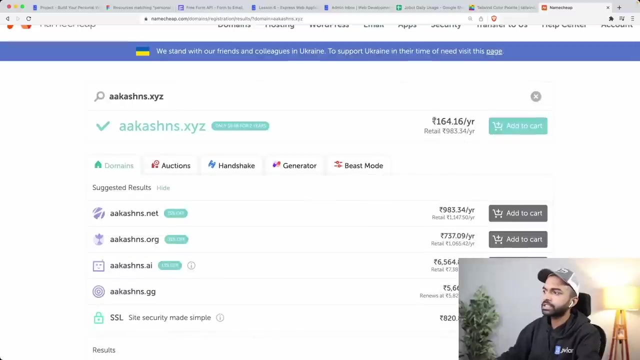 I think some cheap domains are. uh, let's see. So I believe, like dot, X, Y, Z domains are very cheap. So let me, if I, let me just search, for our caution is X, Y Z, Um, I think that's about one, 64 rupees. 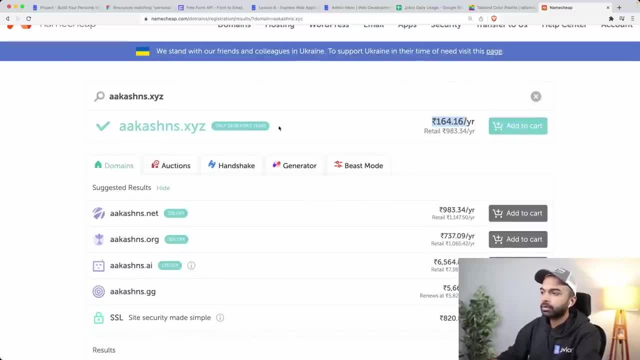 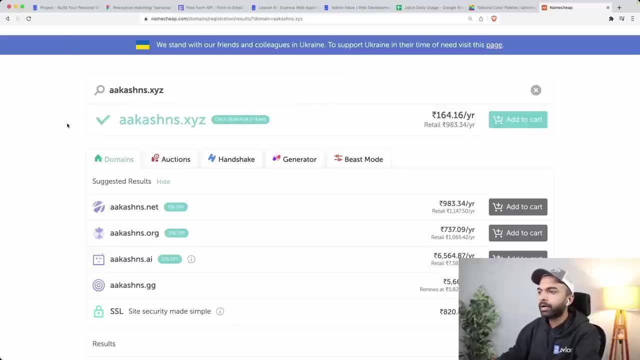 That's about less than $2 a year, right, So $2 a year is not that bad, but, uh, so you can buy it for a bite for a year if you want, but this is not a compulsory part of the um. this is not a compulsory part of the project. 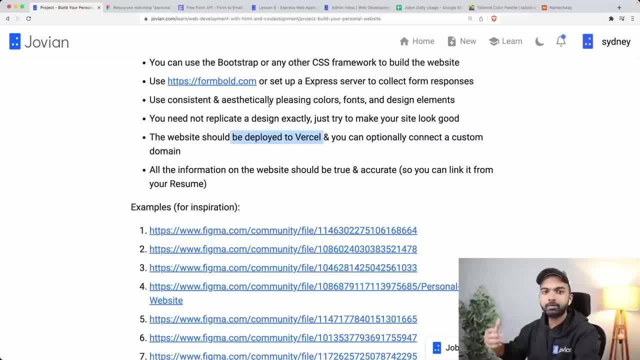 If you know. if it's deployed to Vercel, that's perfectly fine. Even if it's, our caution is dot Vercel, dot app, that's completely okay. No problem there. Now, Uh, one thing I just want. 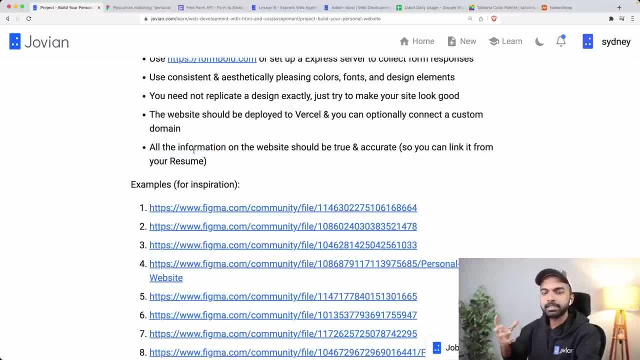 To suggest is: make sure that as you copy over things from different sites, you might find that there is some content there and you might just put that content directly. uh, make sure that all the information on the website is true and accurate. That is key because the? uh, we want you to be able to actually use this website. 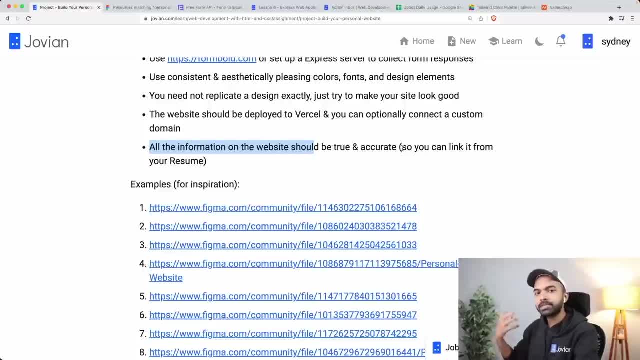 This is not just a project that you're creating. We want this to be a website that you can use, that you can update over time as you work on the uh through the rest of the bootcamp, and you should be able to link it from. 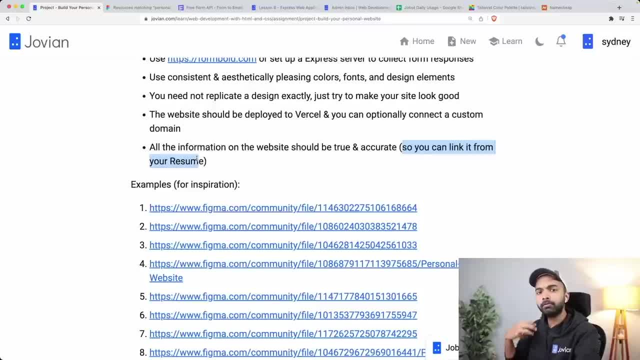 Your resume right. So you want it to be informative for your potential employer, but at the same time you also want it to demonstrate your skills. So finding that balance is the key. here, Again, it's more open-ended. I um, we do not, intentionally, don't want to give you like a set pattern that you can follow here. 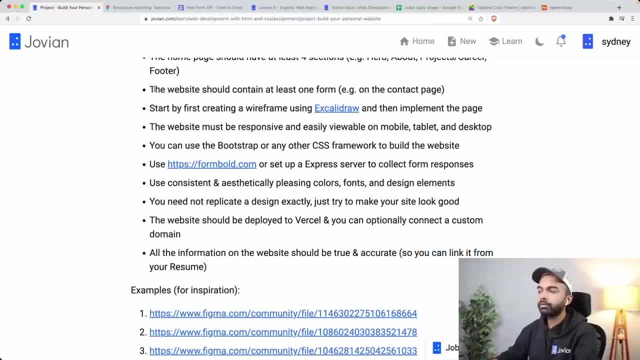 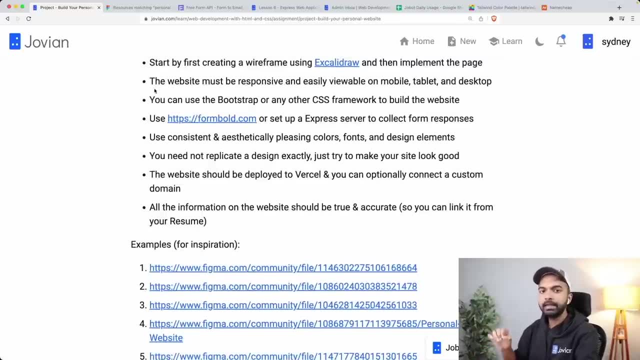 We want you to encounter these challenges. We want you to, uh like, look into these constraints and figure out what is the right balance for you. Okay, And for the project is specifically, I would highly recommend Scheduling at least one one-on-one call, maybe two. 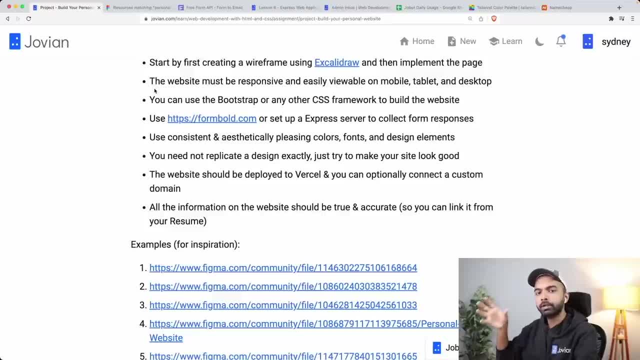 So once, once you, once you've created a wireframe, once you know what your website is going to contain, and once you maybe pick the design as a reference, maybe schedule a one-on-one call just to have a chat, just to kind of go over the content itself. 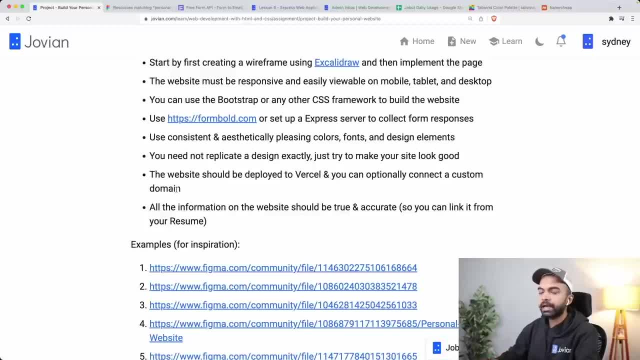 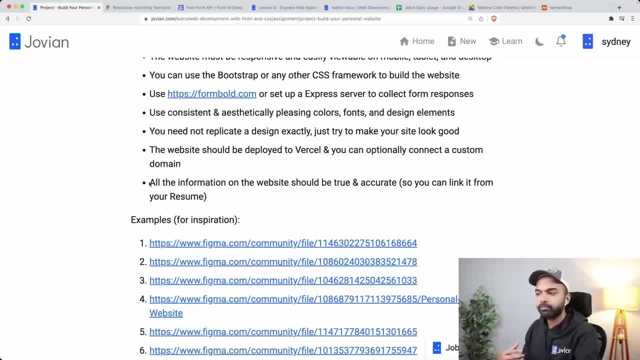 Right, And then the second thing that you should do after that is, once you have implemented the website and made it responsive, maybe you can get one- get on one-on-one call with one of us again to get Inputs on, uh, what further improvements you can make to your website. 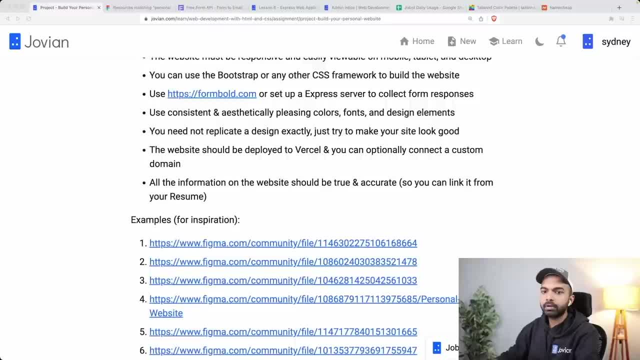 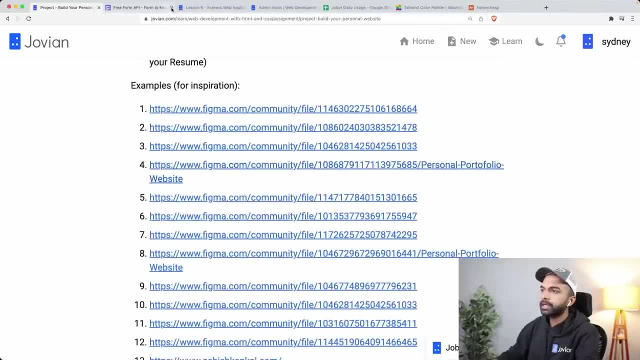 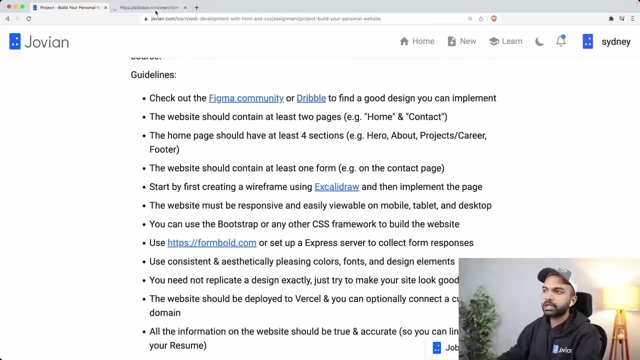 Okay, So those are the two things that I would, uh, that I would suggest you should do. Okay, So here are some examples for inspiration. Let's go over some of these examples very quickly. Um, you can search for more on dribble or the Figma community. just search for personal website and you'll find hundreds of examples. 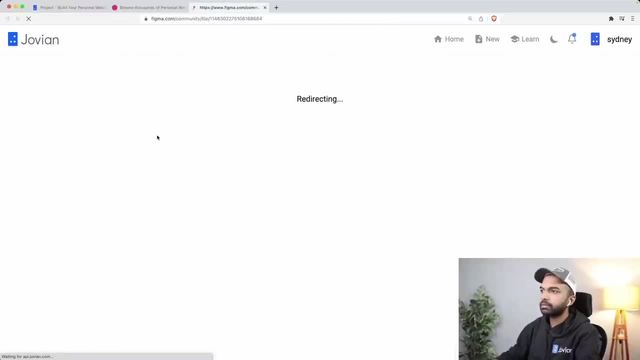 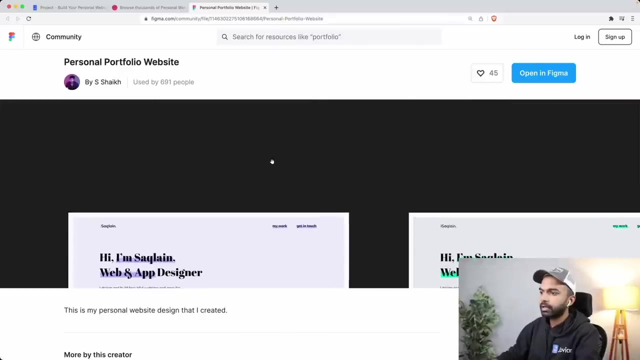 Okay. So let's see, There is this one. This one is: yeah, this one is one that we already looked at, but let's take a closer look at this, So you're okay. It says: hi, I'm suck land. 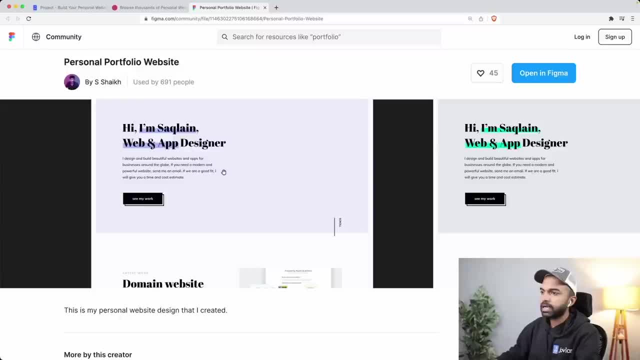 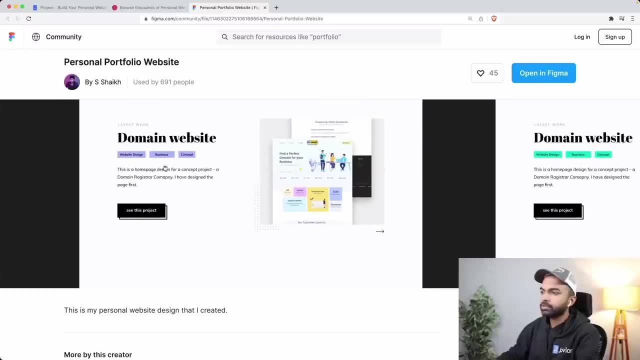 I'm a web and app designer. I designed beautiful websites And of course you can imagine putting a picture here. There's a nice uh um nav bar here at the top, then latest work, So it's put like you can refashion this as an about section. 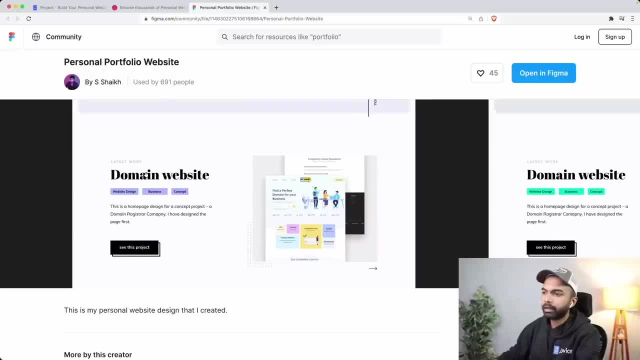 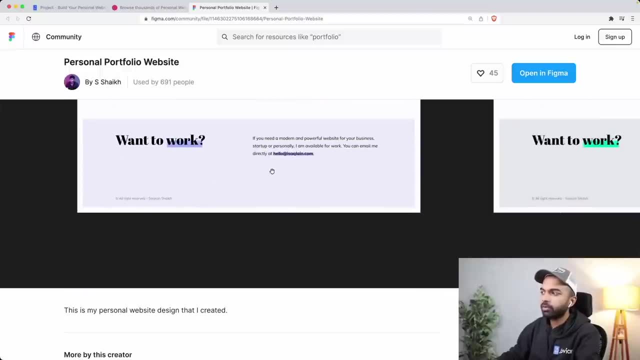 Of course you can just put um, uh about me, and then you can just write a few things here, Uh, and then again, okay, what I do is Okay. So this is more like the about section. want to work. 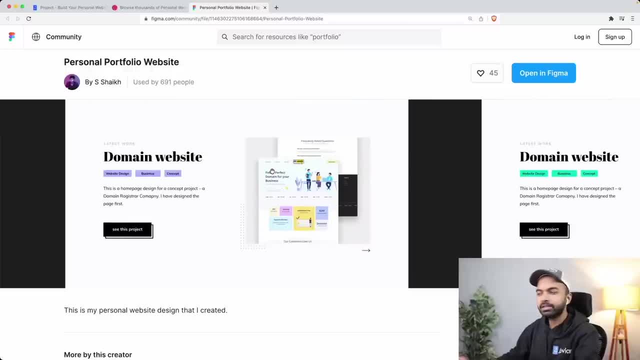 So there's not a lot here. There's like three sections. Maybe you might want to add another section here, or maybe just reuse one of these. Again, this is not- uh, it's not like something that you can use directly. 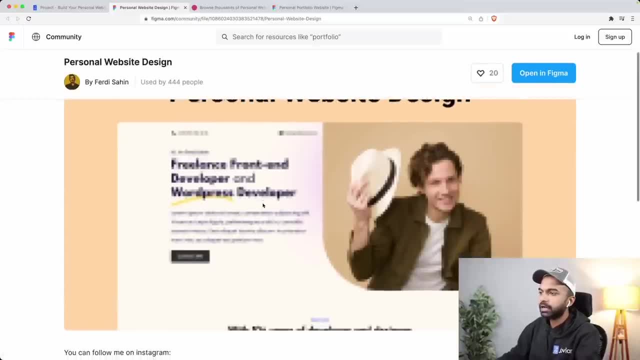 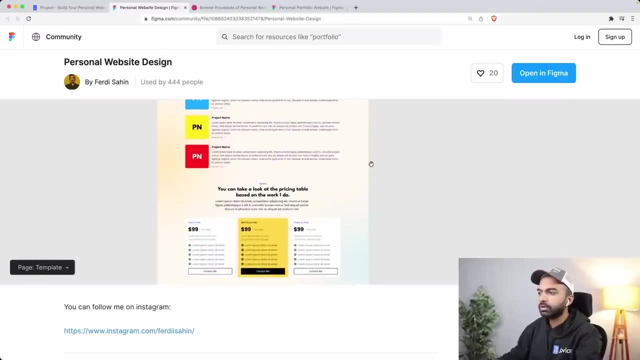 You might have to make slight changes to it. Here is one. This is something that we uh used for assignment one. Feel free to use it If you like it. I would not suggest using this because you will not be learning enough in the process, but this is a good template as well. 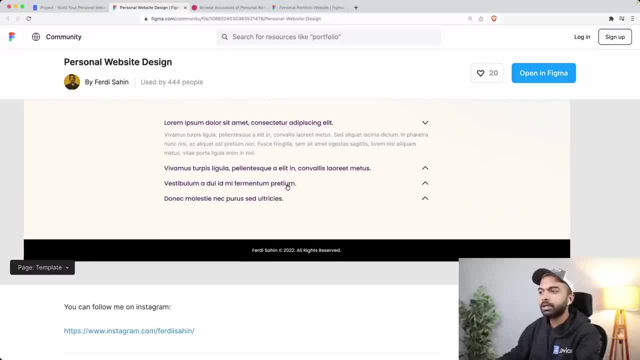 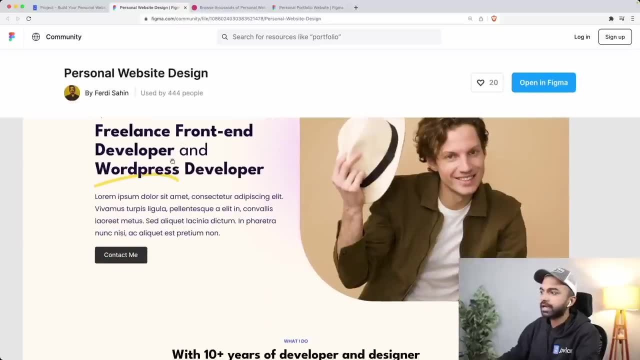 So you can definitely, Uh, use this for inspiration in terms of how to structure your website. If you don't end up using this exact, um, if you don't end up using this exact template itself. Okay, Let's take a look at this then. 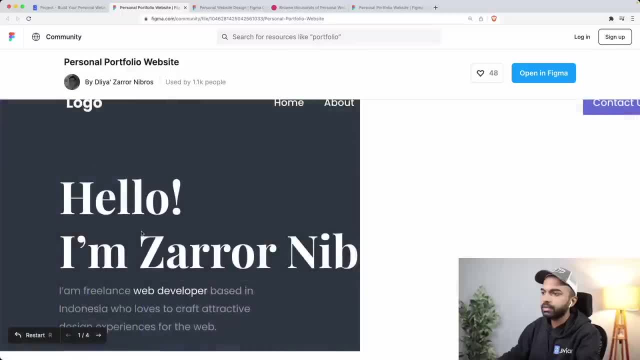 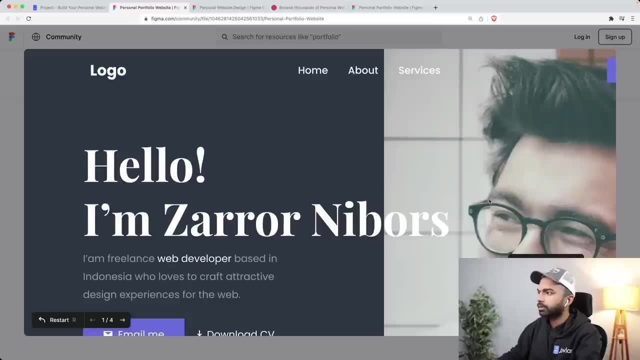 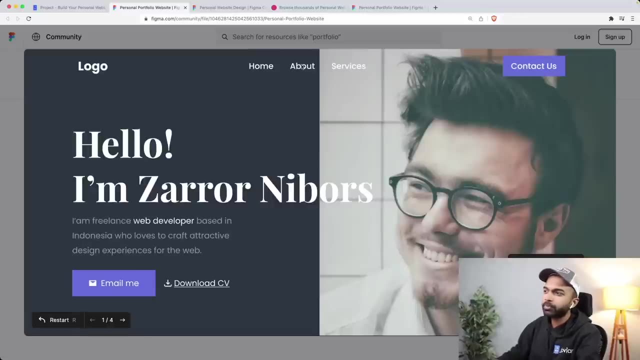 Yeah, This one also looks pretty interesting. It has some interesting fonts as well. So again, let's see. Yeah, there it is. So now you can put a logo here, or you can just put your name here and here. the Napa here is at the in the in the center. 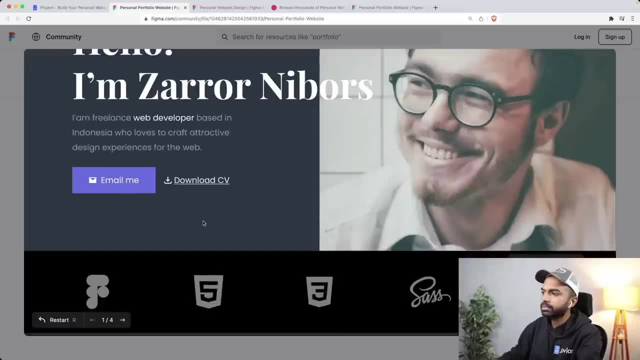 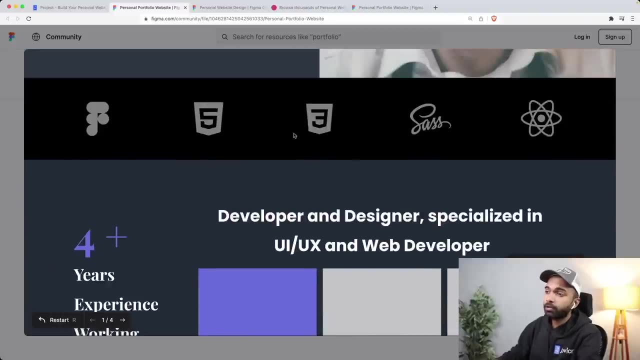 And then there's a contact button. Um then, okay, Hello, I'm Zara. and and then there's some information. There's an email and CV download button. Okay, There are a bunch of logos of uh his favorite tools. 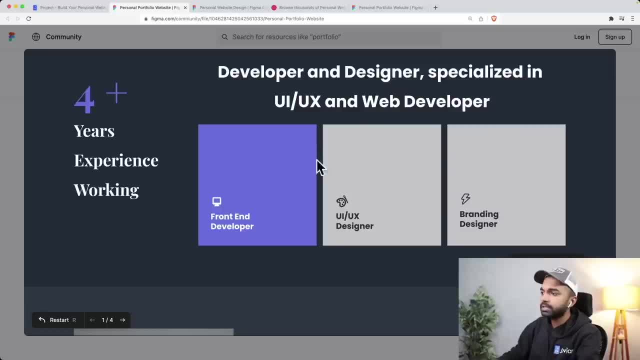 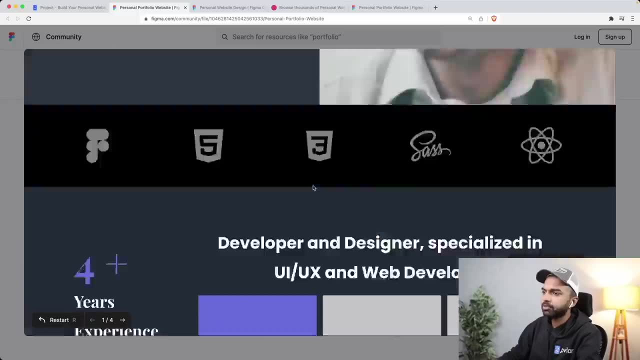 I think that is a good thing. You can put in four plus years of experience and here, okay, There is some information, here There's a code, This could also be an about me and let's connect. Yeah. So four sections. 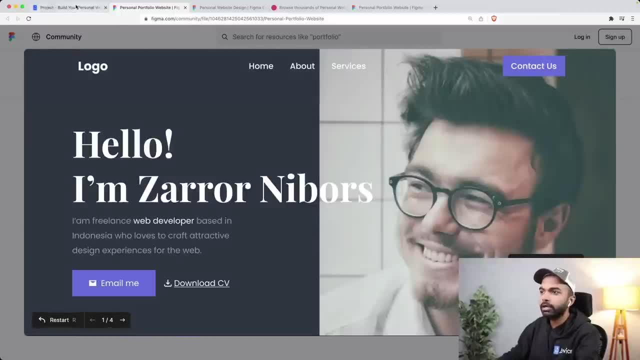 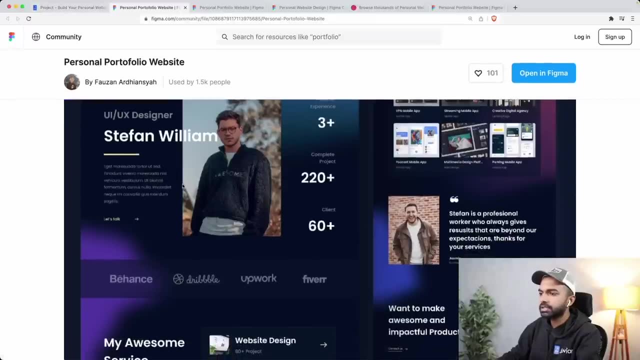 Uh, and of course you may have to think about what content you're going to put here, but again, a good one. Let's see what's up here. Yeah, Stephen William, UI UX designer. Again, there's a bunch of uh interesting stuff going on here. 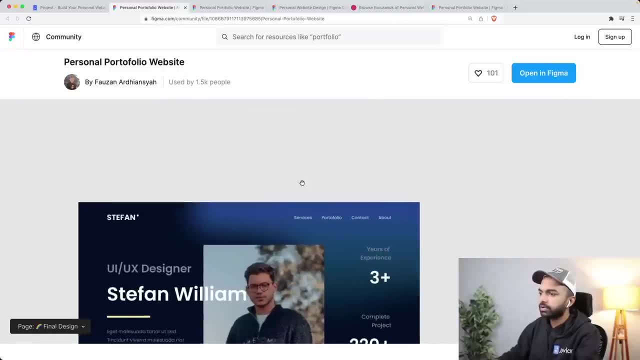 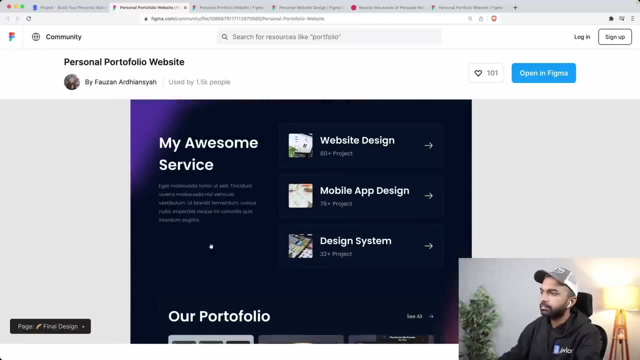 So let's see final design. There are four sections, So there's, of course, a hero section. Um, it has this nice thing on the side That's also interesting then. Um, yeah, these are projects, so maybe you can put some projects here and you can link to them as you work. 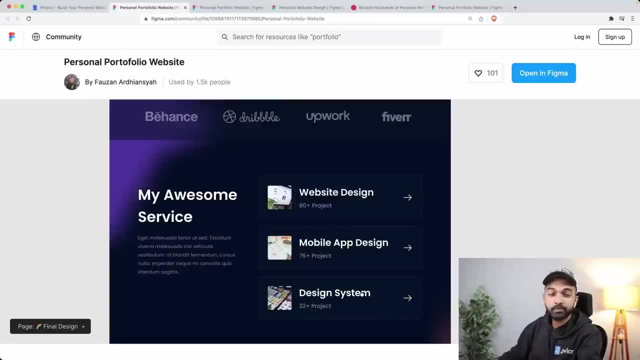 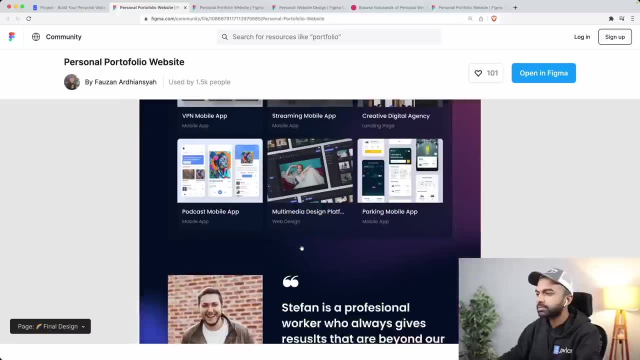 Through the bootcamp. um, you can maybe link to some some of your GitHub repositories here then Okay, These are also like projects, So you could use maybe this one as about, this one as projects or something, And then this one just as a code or something you want to convey to the person seeing it. 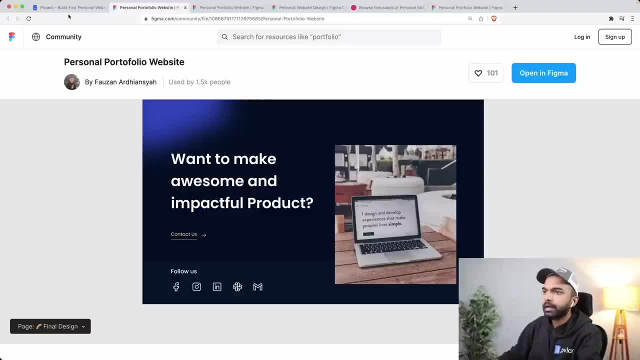 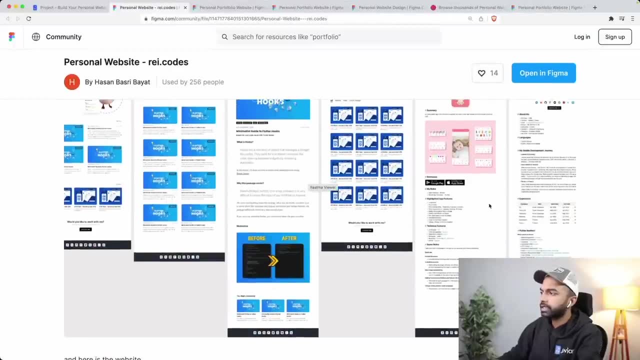 And then this is like the footer, So this is nice. And then let's see a couple more. Yeah, this one is very detailed. You don't necessarily have to use all of these sections, but again, use, Okay, Okay. 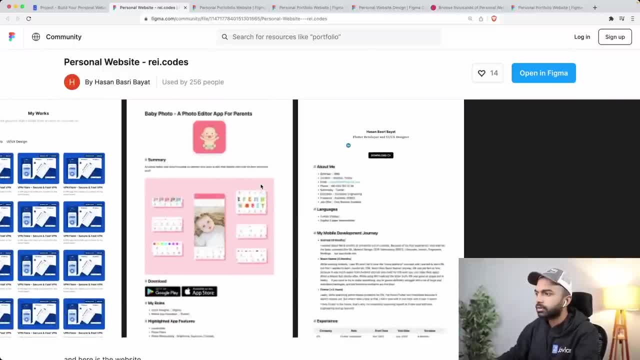 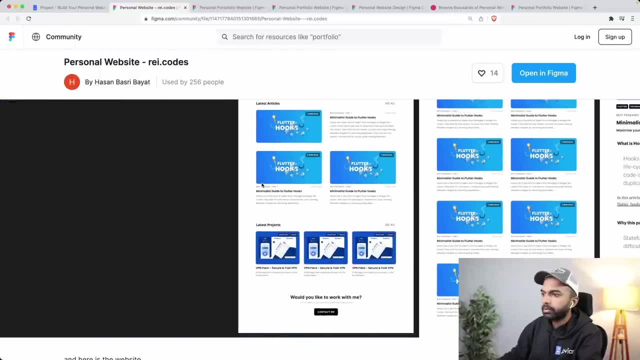 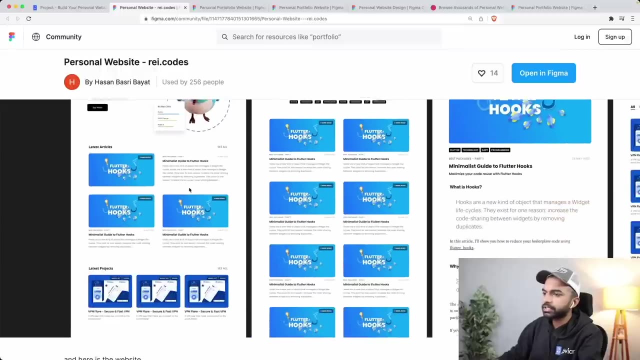 Use it more for inspiration So you can see how it goes. I think this is a great example of how it goes from- um, yeah, how it goes from like a basic design set up here to something that is more interesting here, with a hero section and some articles and some projects and things like that. 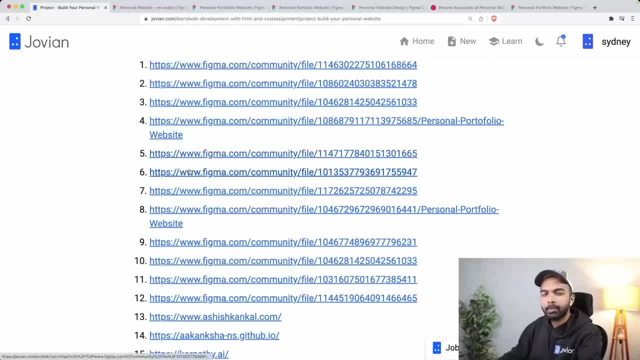 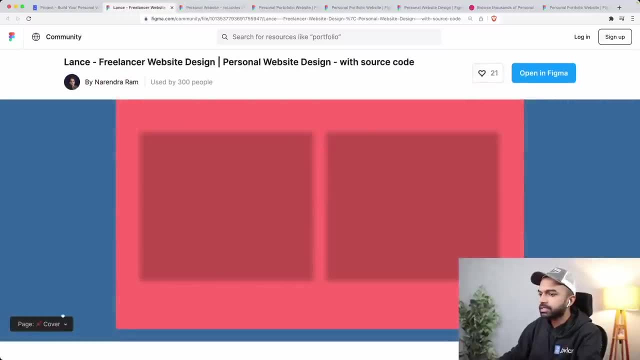 Okay, So great. Um, if you want to add a blog, feel free to add a blog into your website, and blog would simply be a couple of pages. for now, I like this one. This one is really simple. Let's see. 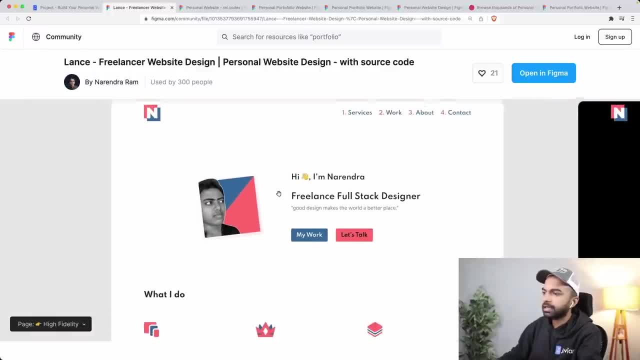 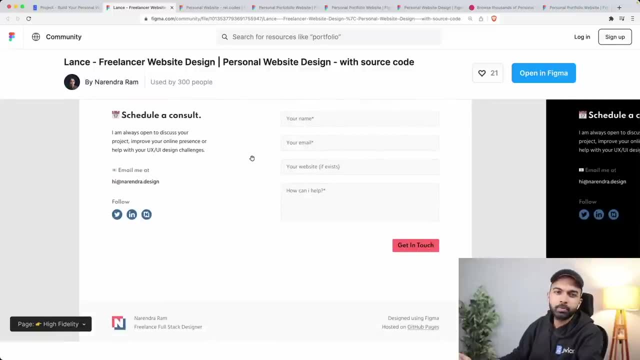 Yeah, So this one doesn't have a lot of images. This is basically this hello section over here And this is what I do: where to find my work, about me and schedule a concert. This could probably go on a second page and that's it. 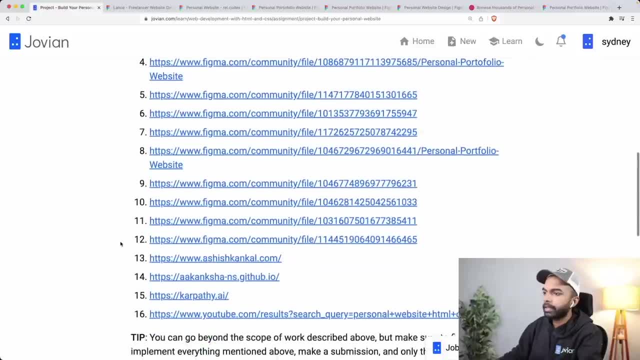 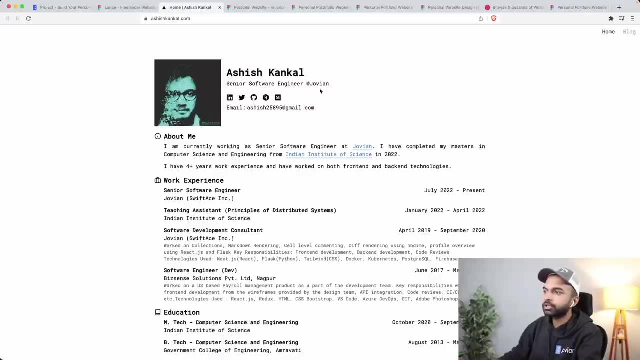 There's this bottom over here, right, Um yeah, a couple of real websites I want to point out. So one you can check out, the website for Ashish. uh, she's a senior software engineer, Jovian again. 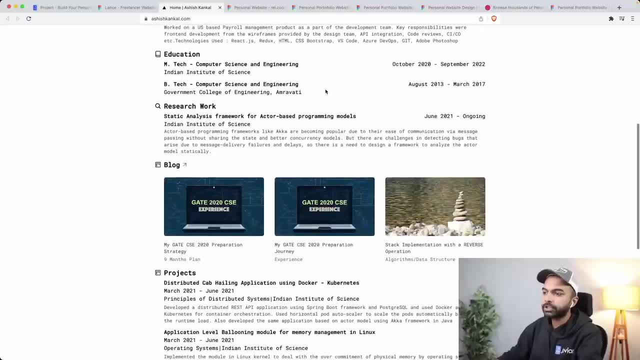 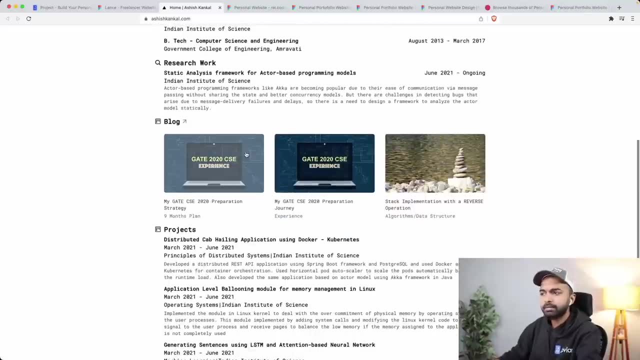 This is a. It's a very different style and this is a sort of a very minimal approach here, but I think it covers everything. Uh it, it has a. it's very text heavy. It's sort of more structured like a resume, but it's great. 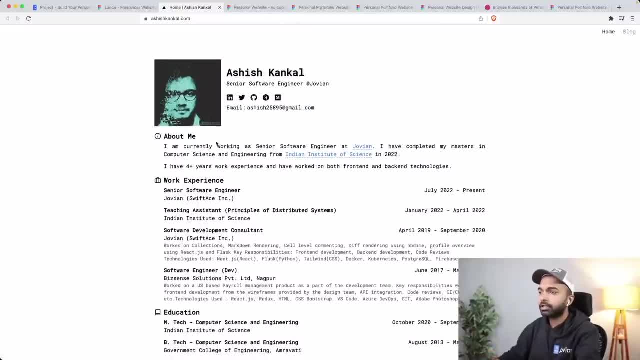 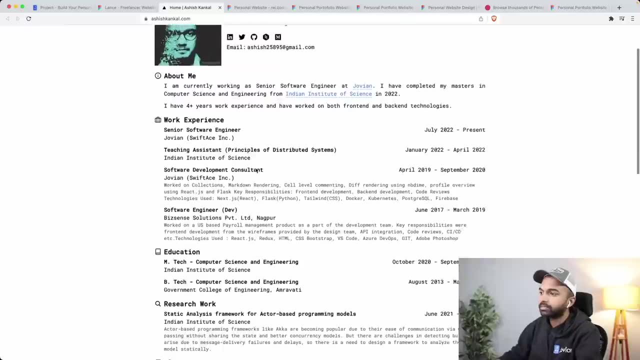 It does the job And for a developer it actually might be a good thing. The font used here is a mono space font, So that's again an interesting choice of font. Um, but again, for a programmer that is something that might make sense. 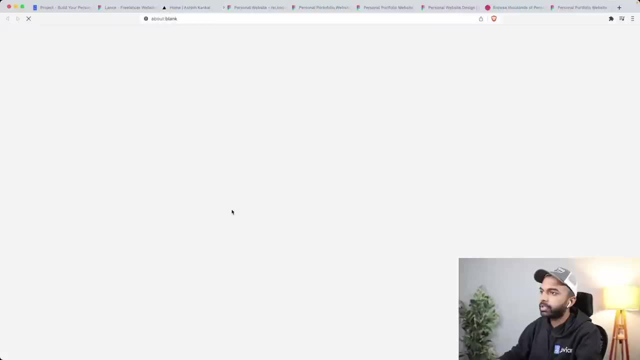 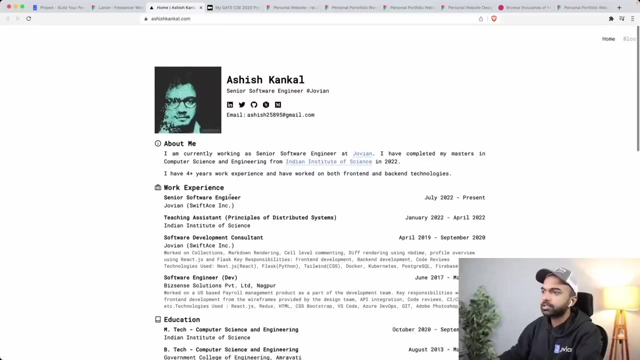 And then there's a link to a blog here, And then so again these, these open into different, uh, other websites. So That's fine. There's a project section, There's an achievements- Yeah, So this is more structured like a CV and that's perfectly fine. 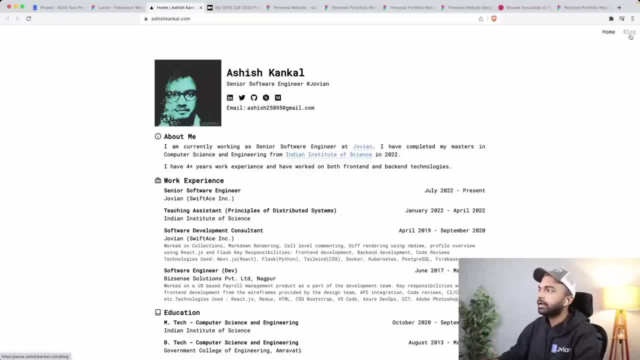 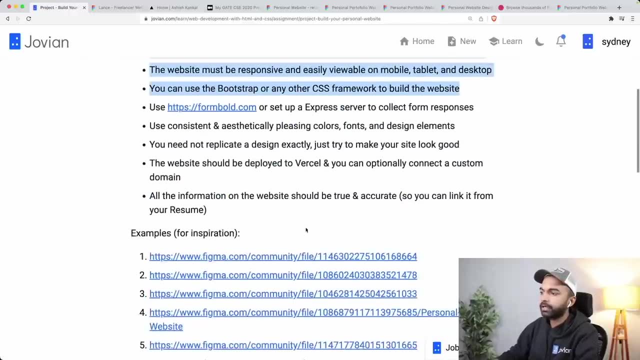 It's your personal website. You give it your personality. Uh, just as long as you are satisfying the requirements that we have laid out here, that is perfectly fine. Here's another personal website you can check out. Um, so, this is Akansha. 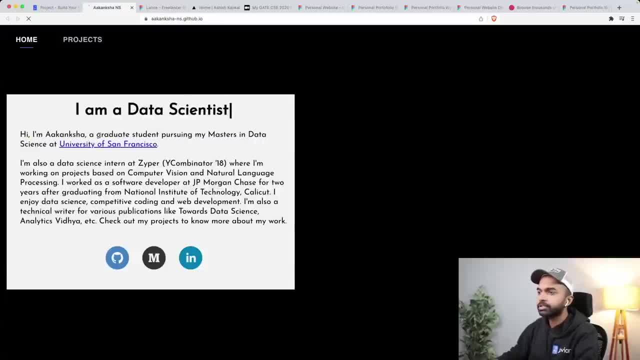 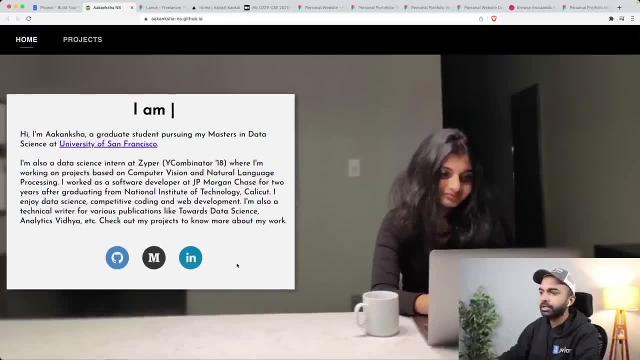 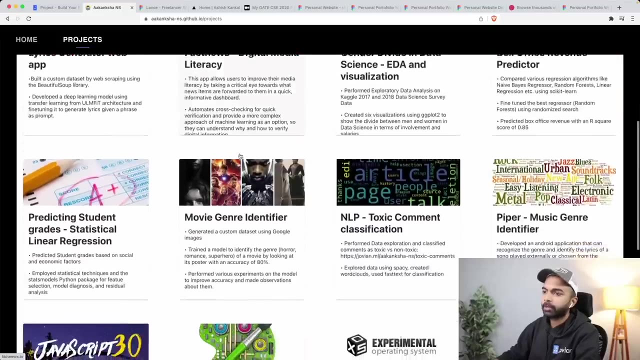 She is, or was, a graduate student pursuing masters in data science. So here she has a home Home page where she has a picture, she has this, uh about section and uh, she has a bunch of links. and then she has a project section where she has like a bunch of cards, uh, showing her projects. 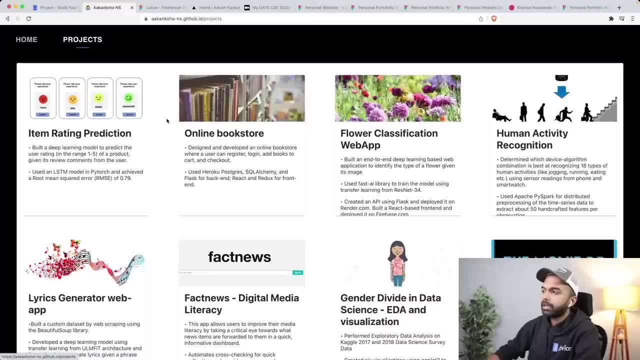 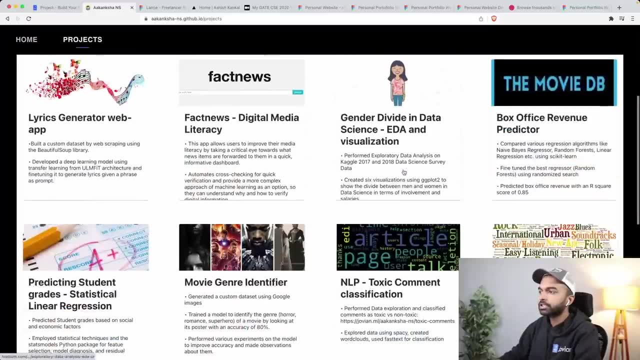 Right, And this is great because it um it. it simply shows you that, okay, you go to the site, you learn enough about this person and you can go into the project section and then you can check out: okay, this person has done a lot of interesting work. 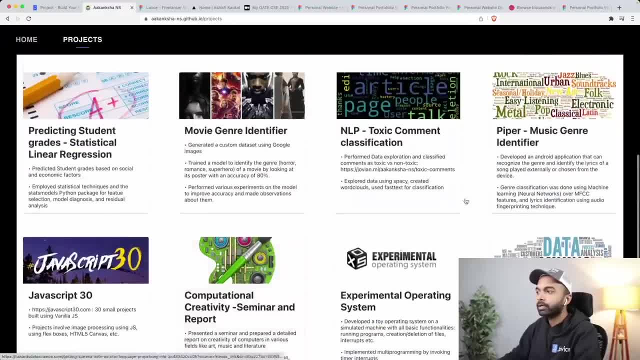 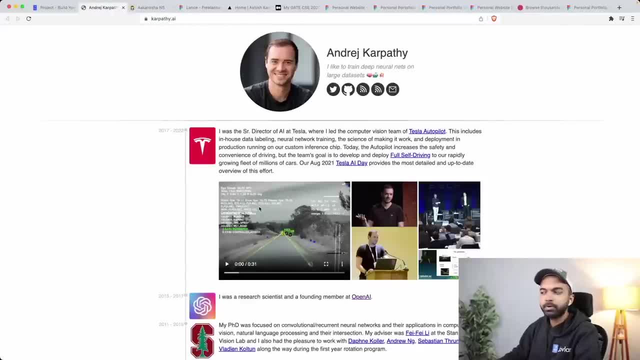 And I probably want to like, as a potential employer, I probably want to talk to this person. Then, um, here's another one. another, like a lot of people, take a more text heavy approach, and that's perfectly fine. Again, I want to stress that this is your website. 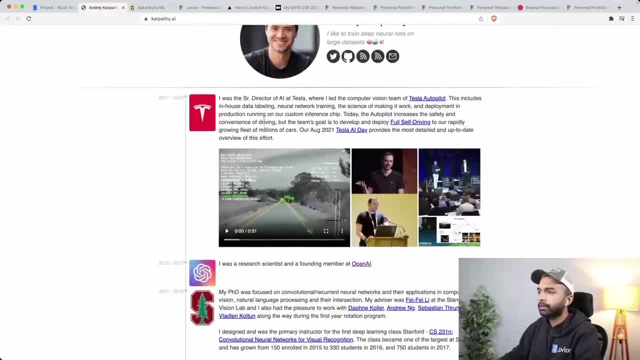 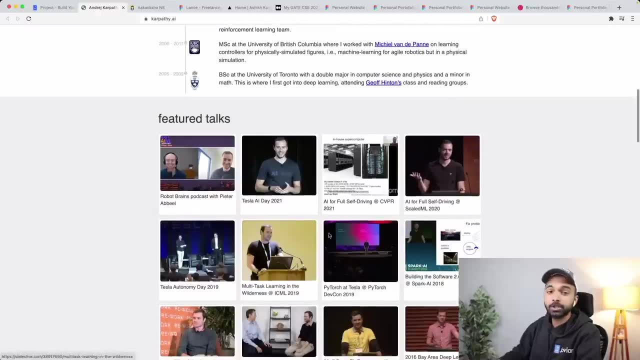 So this is Andre Carpati. He's a researcher at open AI Um, so before that he was working at Tesla. So he has this simple website where he has a timeline of his work, And after that he has some featured talks or um that he has given over the years, and then a little section about teaching, a section about writing. 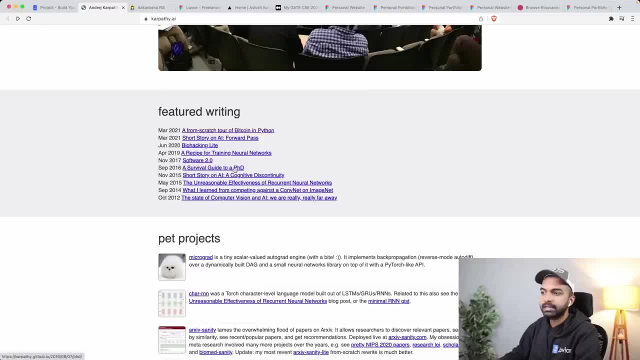 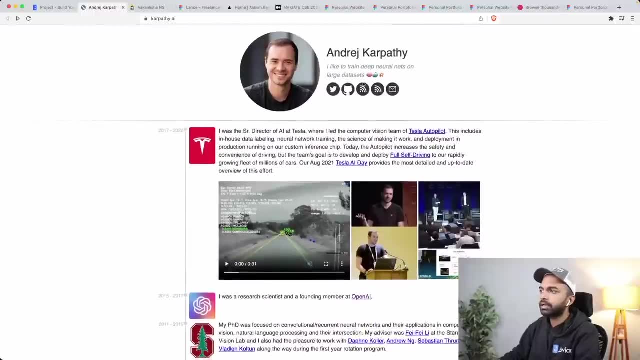 Uh, and in this case, yeah, the right. the blog actually opens on a Different side, And that's perfectly fine. A bunch of pet projects and publications, et cetera, Right, So again, great, It's all. and then the bunch of social links here as well. 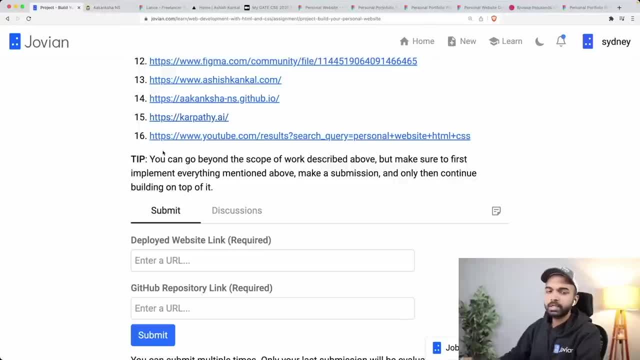 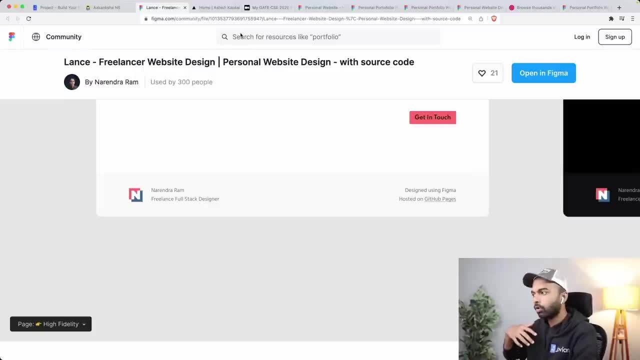 So perfectly fine. Uh, this works too. So I want to say that don't limit yourself to the kind of websites that you see on Figma or on dribble. uh, go, feel free to go a little um wider in terms of your search. 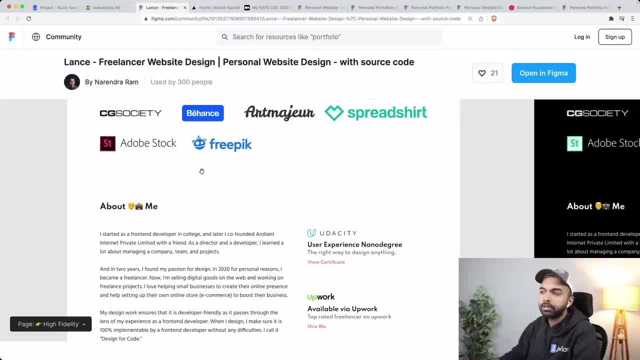 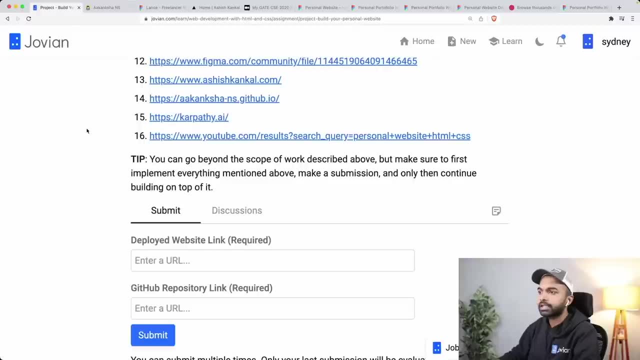 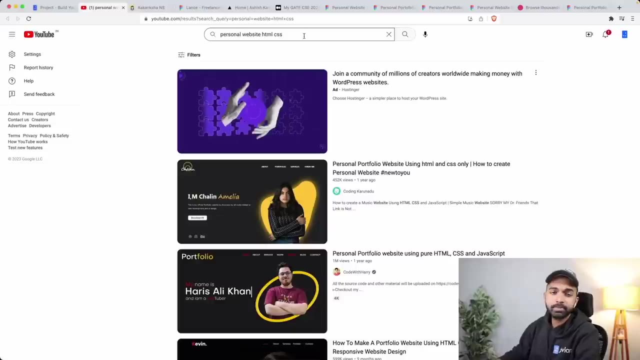 Feel free to just look at personal websites of people Uh you generally tend to follow. you can generally find them on their Twitter. You can find them on their uh, on their LinkedIn for project or elsewhere. One other good source for a bunch of these sites is just going on YouTube and searching personal website HTML CSS and you will find your. okay, this looks interesting. 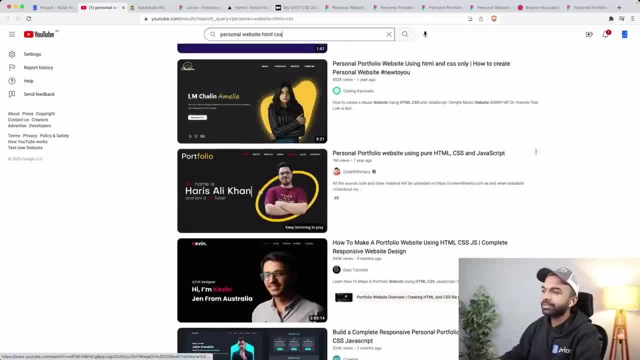 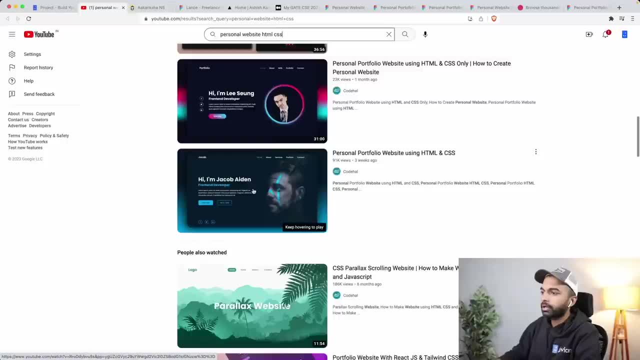 That looks interesting. That looks. these three look somewhat similar, I would say, but still, uh, this looks pretty interesting. This one, uh, this one over here is also good. Um, yeah, this is also interesting. This has got some. this one looks pretty slick. 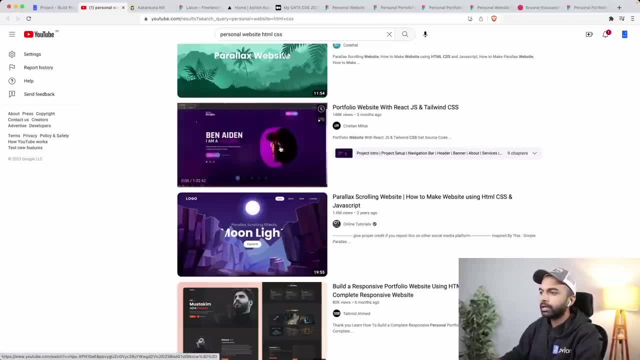 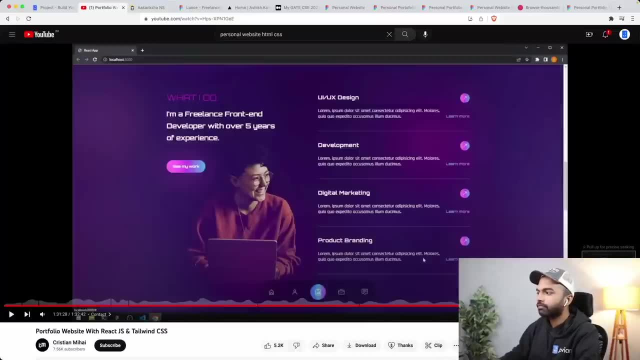 I mean, it's got that whole cyberpunk team going on and uh, it's also a tutorial, So you can actually probably even follow along with this. And again, it's fine if you are uh referring to a tutorial a little bit. 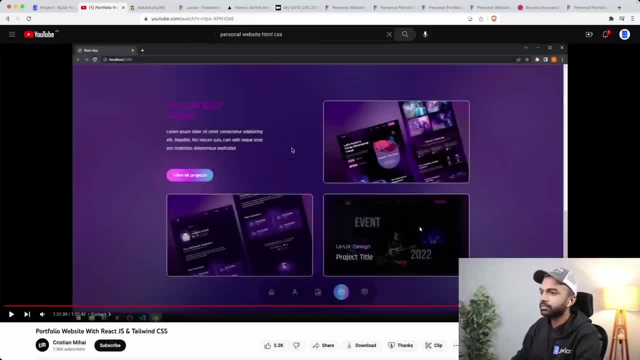 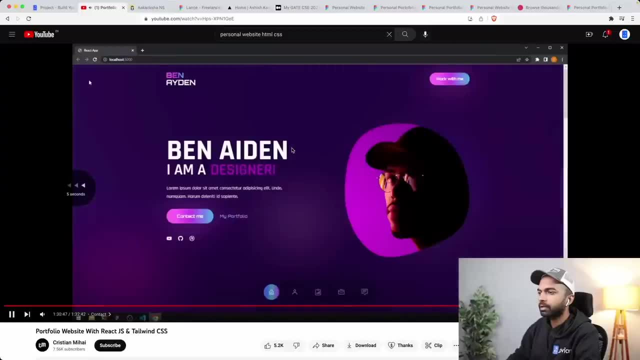 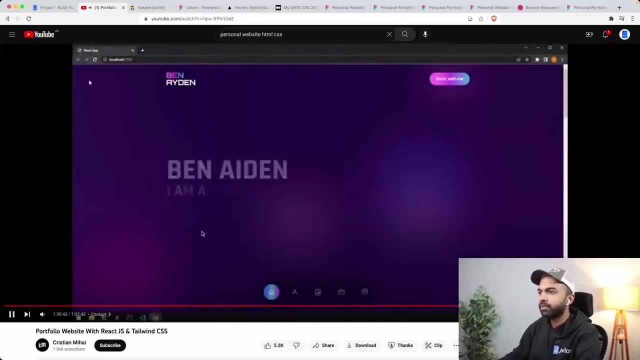 So let's take a look at this. This one's got- uh, got a few animations as well, So let me just play this. Yeah, So this is what this website looks like at the end of all of this. So this development, I believe this is implemented in react, but it doesn't have to be. 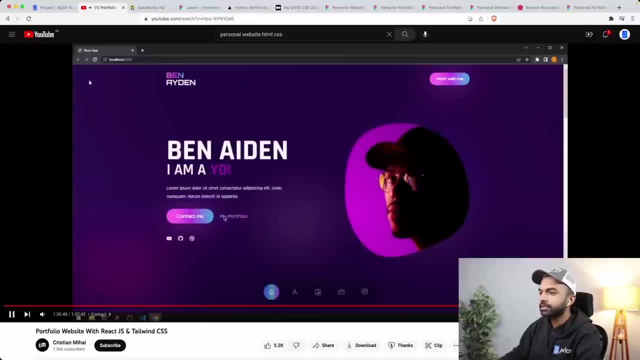 So it's got a bunch of animations. It's got it's got a bunch of colors over here. It's got this nice bottom sticky bottom bar. Um, let's just watch the entire demo over here. It's got a portfolio link. 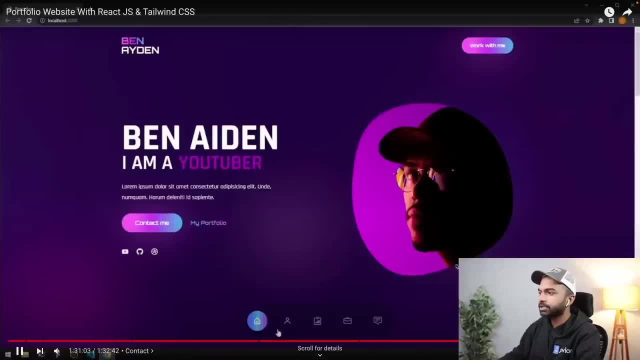 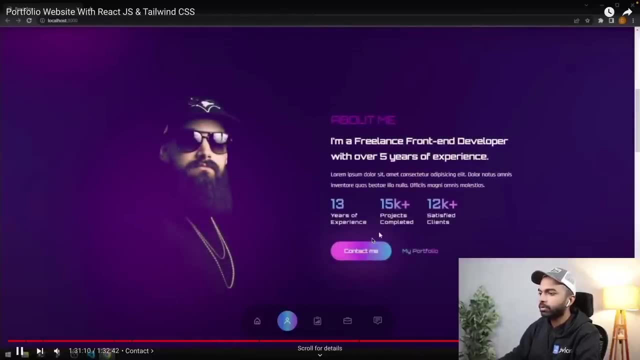 It's got a bunch of social links. It's got this nice image which is cut out in a random shape over here. Got this nice about section. There's some Uh animation going on Here as well. there's an animation on the buttons too. 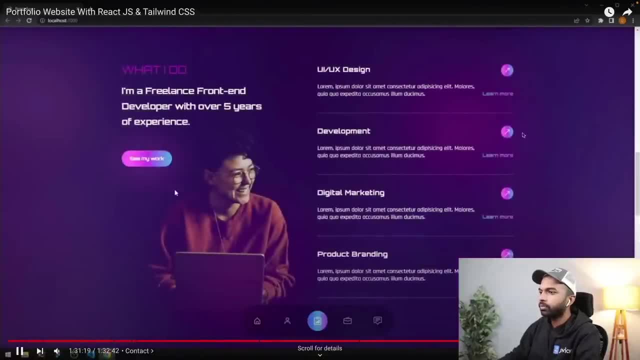 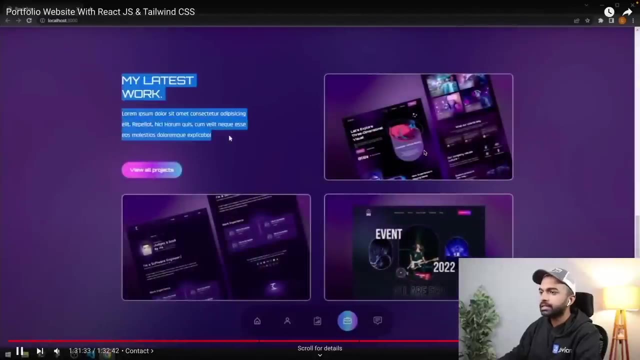 Then there's a more detailed section, What I do. again, this could be projects as well. possibly. Let's keep going And yeah, these are like some latest projects, so that and then probably there's at the end, I believe there is a contact form somewhere. 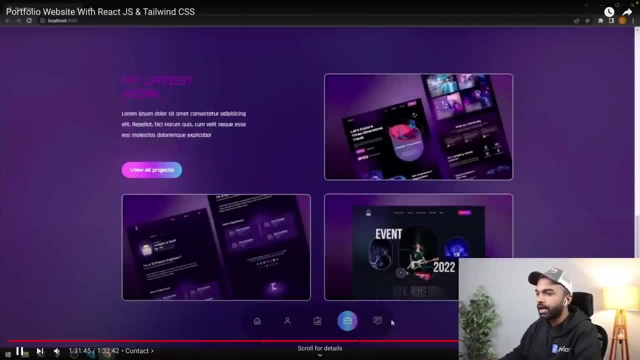 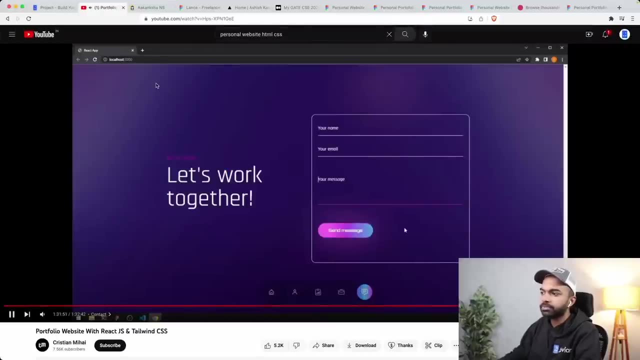 Yeah, So again, you don't have to add any animations, but if you want to, you can and um, there are often you can use a bunch of like CSS or JavaScript helper libraries to implement animations. Bootstrap itself also allows you to create some animations. 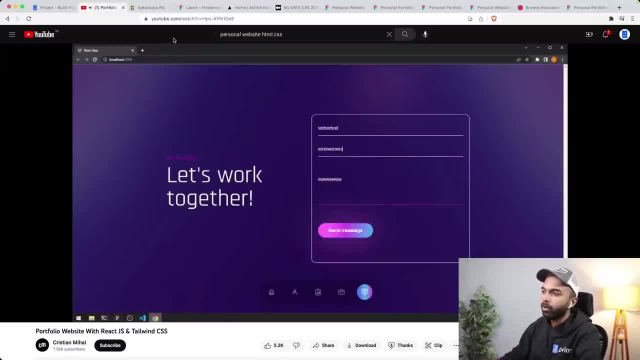 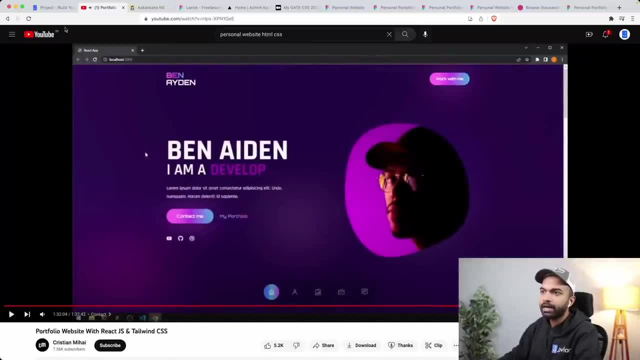 The reason we don't cover animation a beginner course is because most websites will not require any animation or you'll end up just using some pre-packaged library. but if you want to add animations, please feel free. Uh, we're not stopping you. 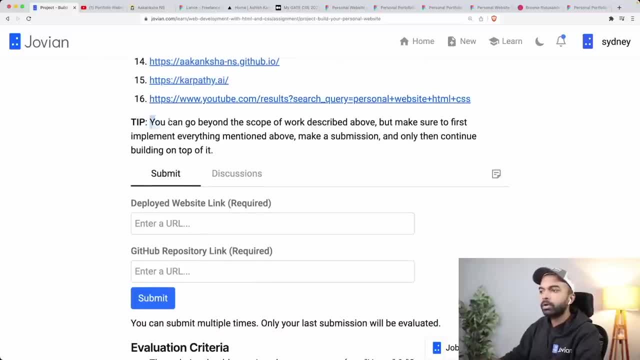 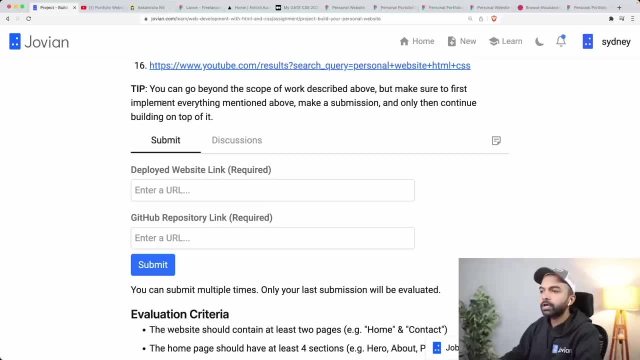 So one tip I want to give you, a very important tip, is That you can go beyond the scope of work as, uh, that is described above. You don't have to limit yourself to this. However, make sure to first implement everything that we've mentioned about. 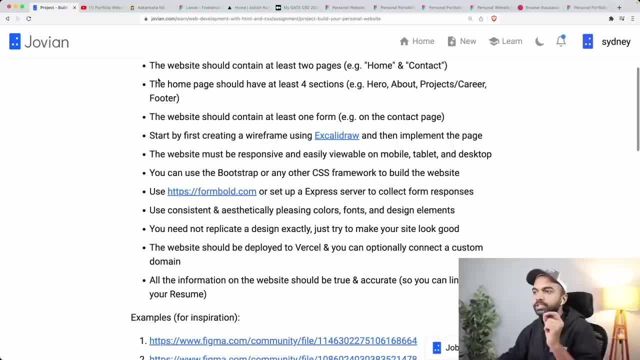 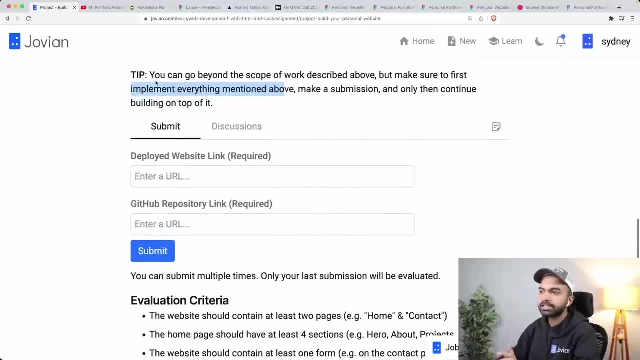 So first do a first pass and implement just the bare minimum. just implement everything that we've done before going too heavy on, let's say, creating five pages and all that. So first create a basic version that satisfies the evaluation criteria, make a submission here and only then continue building on top of it. very important. 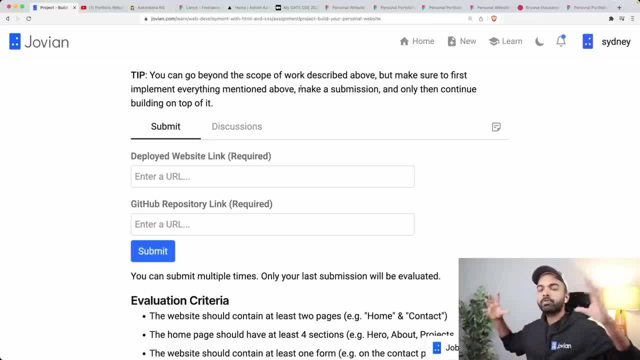 You have to do this iteratively, Because If you keep expanding the scope of your website, you will be stuck on the first page or the first section forever And you will never actually and you will be trying to animate the first section, the hero part of it and all that. 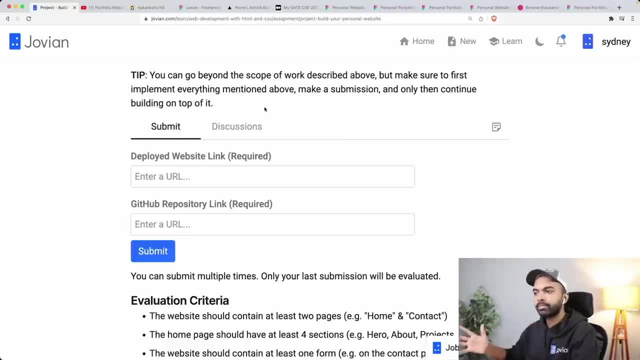 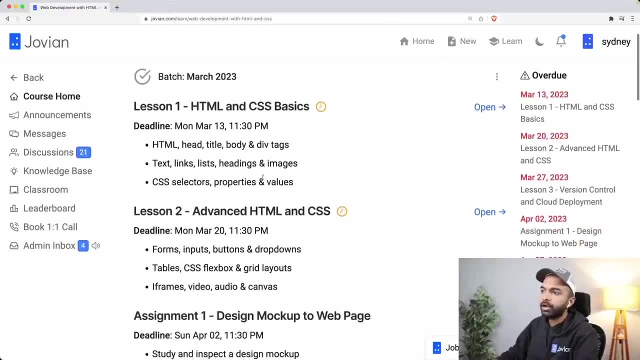 And you'll be just stuck on that for days, right? So do the basic version, make a submission. We'll give you feedback as well, Um, and then continue adding whatever else you want to add. Okay, Uh, we started out by looking at HTML and CSS basics. 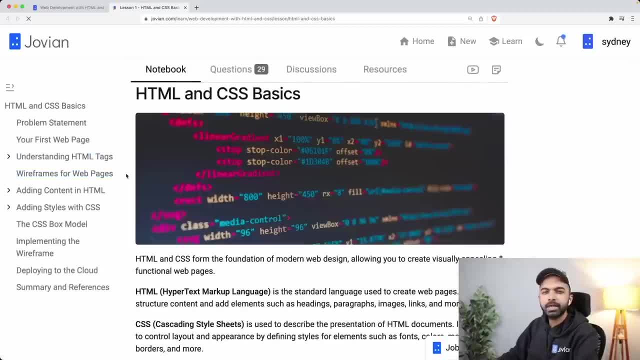 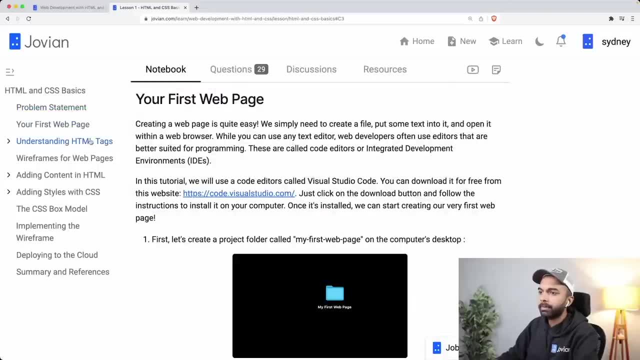 Um, so Yeah, we just understood HTML, CSS, The very basic Foundations of, uh uh, web development. So we wanted to create our first webpage. and creating a first webpage, What we really wanted to do was we wanted to create a Jovian jobs website, which 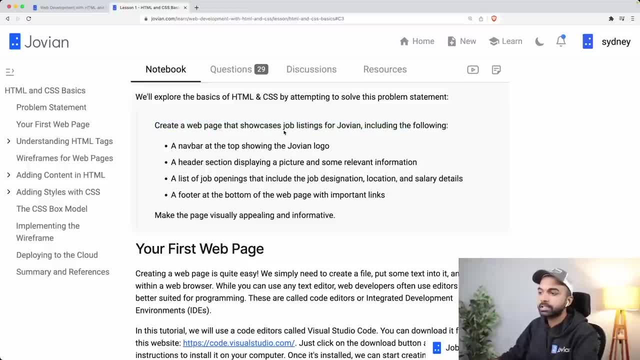 we kept building and improving over the course of, uh, the several lessons And we just wanted to have a nap bar a header section displaying a picture, a list of job openings, and a footer at the bottom. uh, and that for just for. 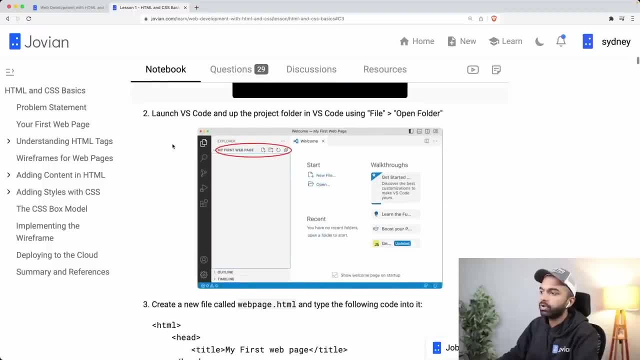 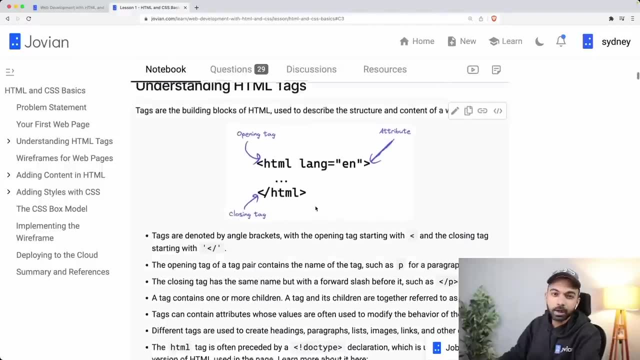 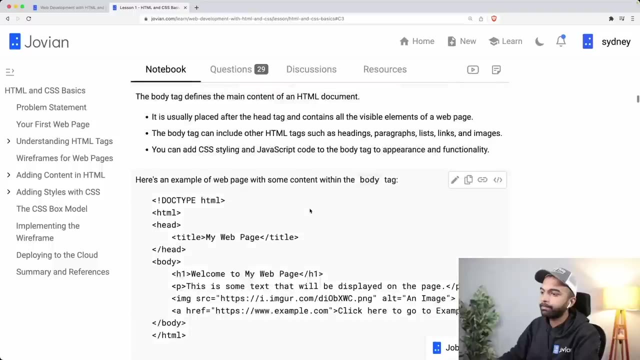 that what we did was we uh created a folder on our desktop, We opened up visual studio code, We added just some HTML code to it. that showed us our first web page, And then we understood how tags work. Then we uh created some important tags like HTML, head, body, title, et cetera. 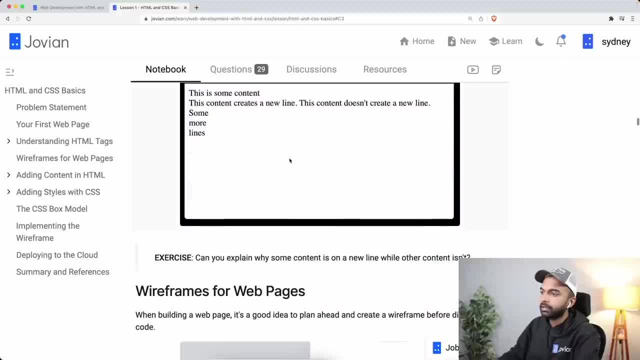 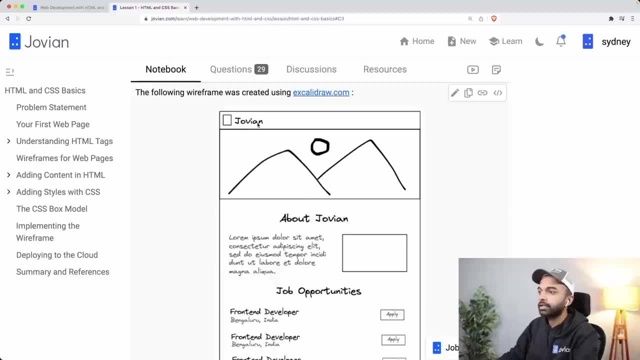 Then, uh, we added some div tags with some content. Um then we had created a wireframe. So we decided that, okay, we need to maybe first create a wireframe like this. So this is where it all started. Uh, okay. 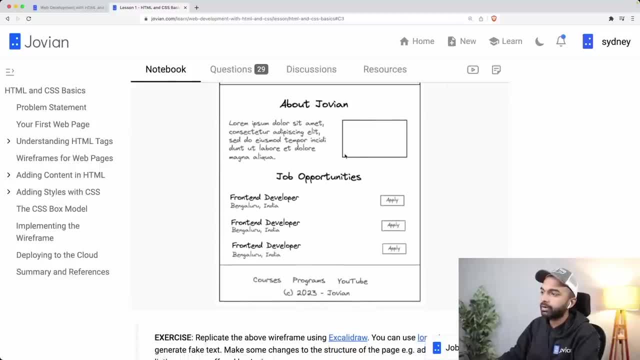 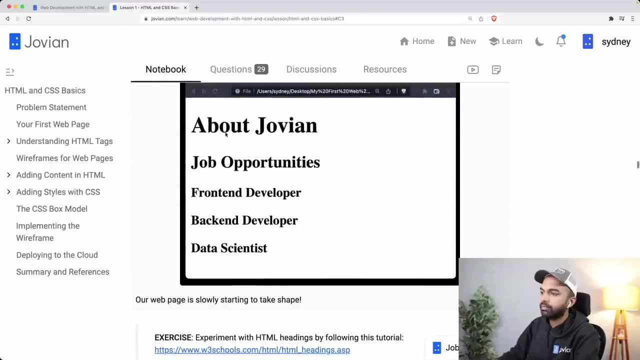 We wanted to have a nap bar. We wanted to have this header image. We want to have an about section job opportunities and a. Then we added some content, uh, using HTML. So again, we added a bunch of headings like this: 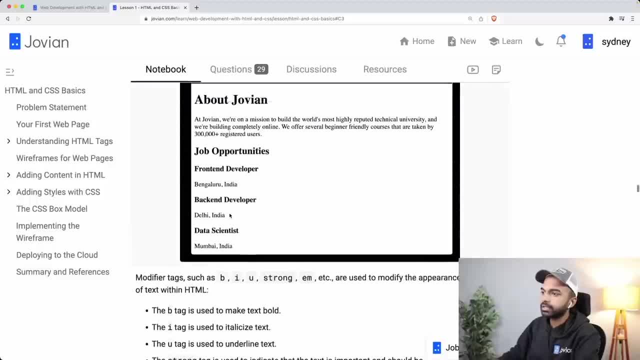 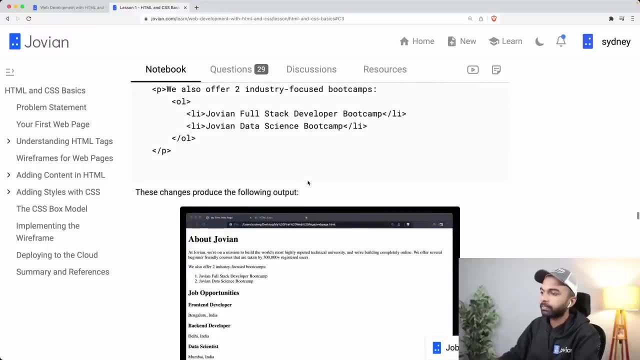 Then we added some text and paragraphs. So then start, things started looking a little better. Of course, it's still basic content. Then we added some lists, So we created a list for- uh, let's see, we created a list here, an ordered list. 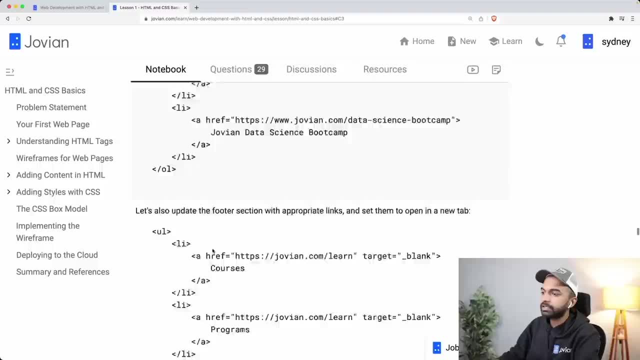 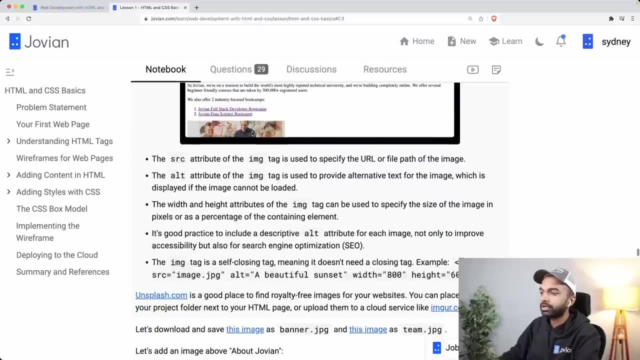 and an unordered list here for the footer. Then we added some links. So, after adding some links, this is what our page looked like. Then we added some images. So we added an image- Okay, Share- at the top and image here below. 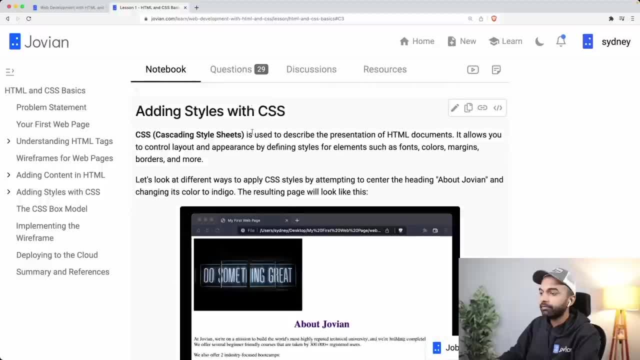 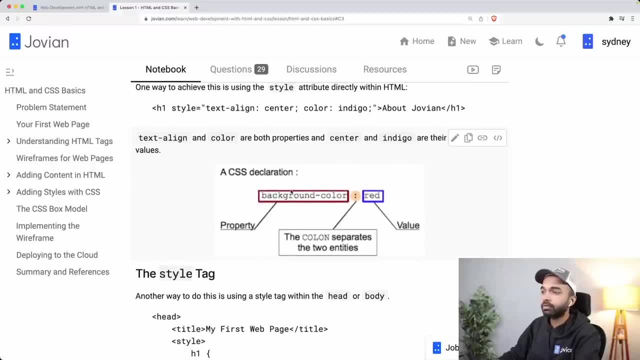 And, uh, this is what our page looked like without any CSS. Then we went ahead and added some CSS, So we started centering things, We started adding some image styles, So we learned how CSS declarations work. We have some selectors and then we have a property and a value and we 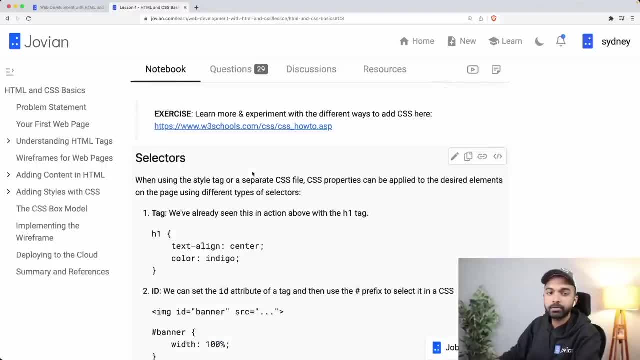 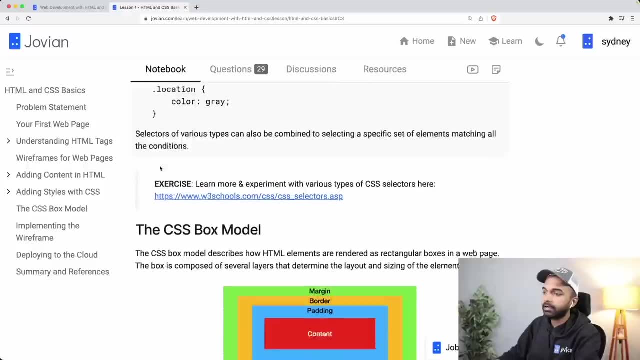 can put it inside the style tag, We can put it in a CSS file or we can use the style attribute. Then, uh, we looked at the different ways to select a tag and ID a class and we understood the CSS box model where we have some content padding border margin and 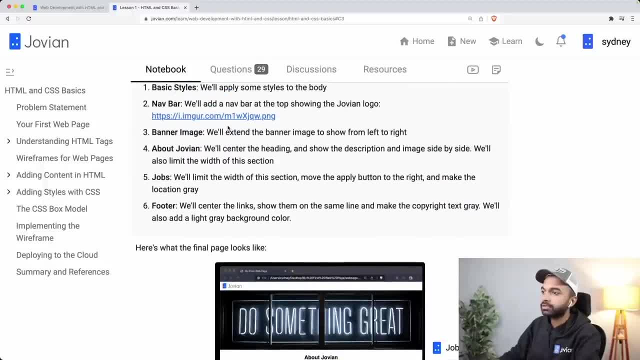 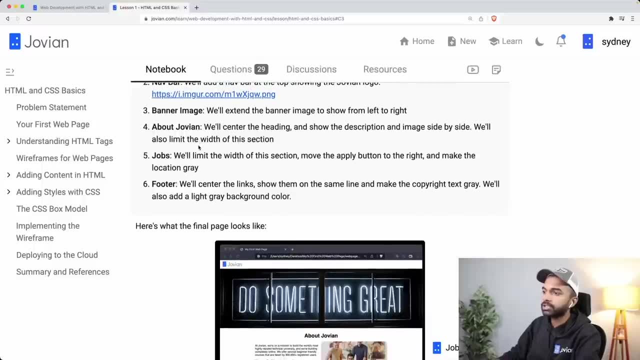 then we implemented the wireframe. So we started by adding some basic styles, So just adding styles to the body, then adding the nav bar, uh, with a Jovian logo, then adding the banner image, the about section, the jobs, the footer. 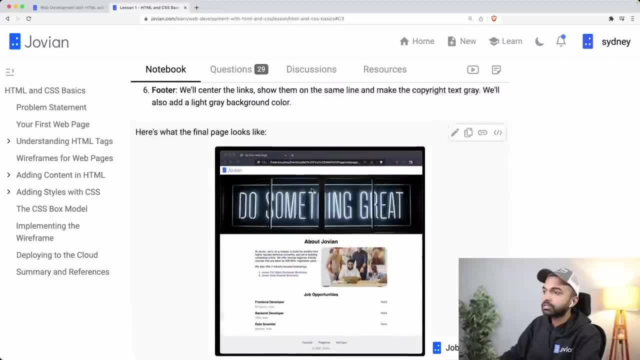 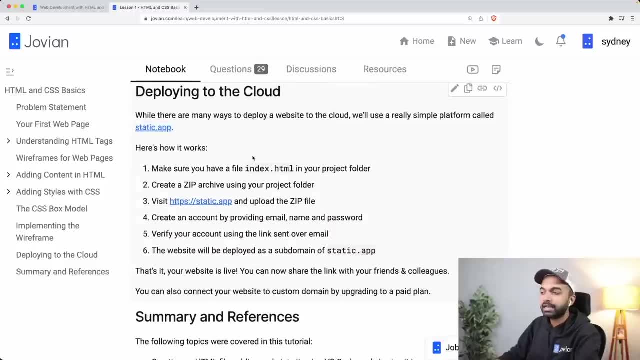 And this is ultimately what our first web page looked like, right? So once we did all of that, this is what our first web page looked like, And then we deployed it to the cloud using this platform called staticapp- Not something that you would do. 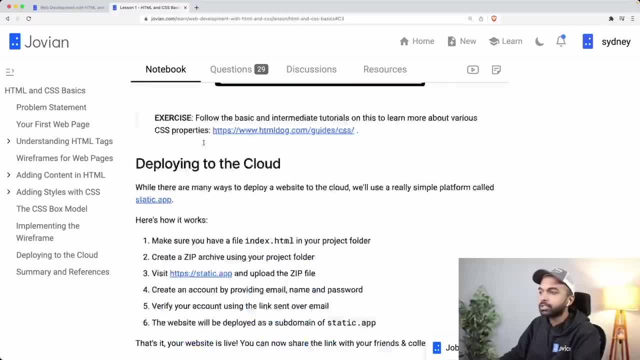 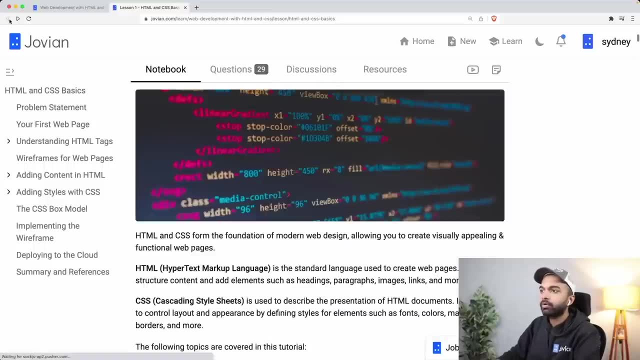 In production, but it works for our first web page, And that was that was our first web page, And that was not too bad for our first web page, Uh, but this is something that we then kept improving on over the next several lessons. 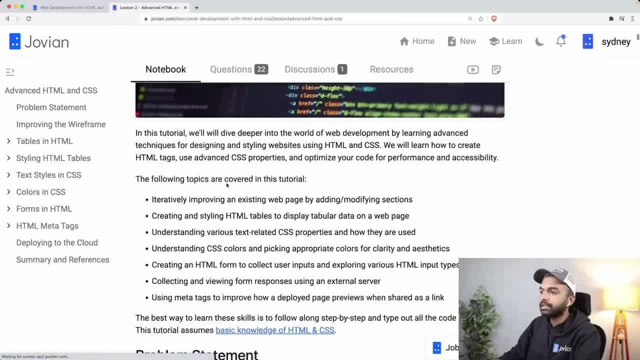 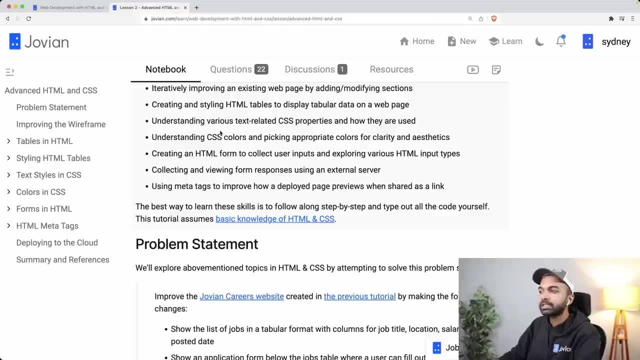 So in the second lesson was advanced HTML and CSS, And this time we just wanted to iteratively improve the existing web page by adding and modifying sections. We want to learn how to work with tables, how to add forms, how to and how to work with colors in CSS. 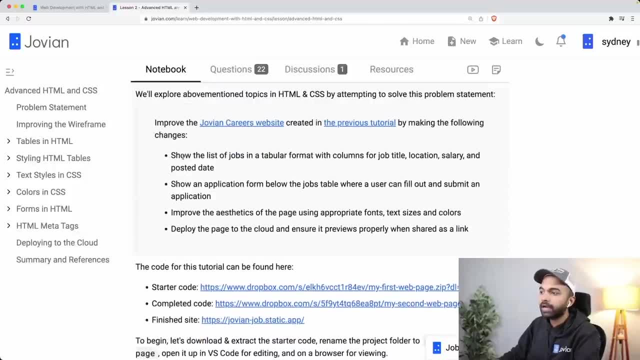 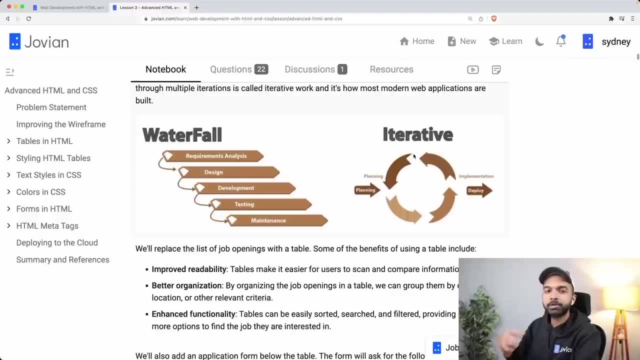 How to um save, how to use meta tags, all of that. So, again, we basically just and we learned about the iterative method, and this is something that you should try to apply to your own personal website development as well. 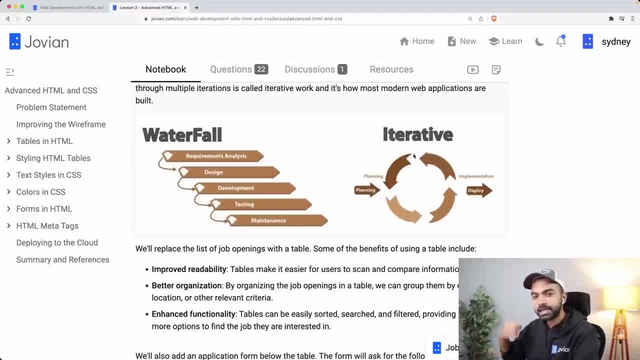 Try to get the first version out in one day and maybe then take the second version out. Everything is something that should be deployed, And that is why we may we also focus on deployment from the beginning. Your website should be live from day one and you should just keep adding. 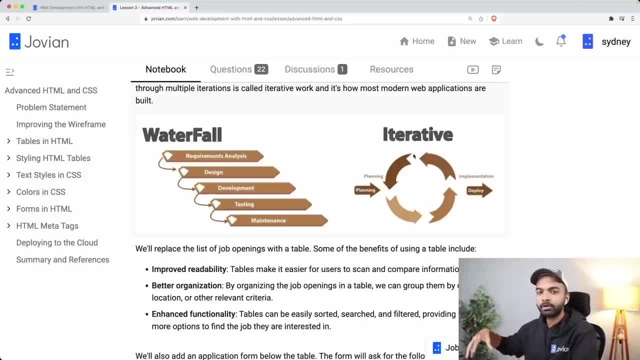 more information to it instead of saying, okay, I'm still working on it, I'm still working on it, I'm still working on it, I'm going to. I'm going to put take it live tomorrow or next week or something like that. 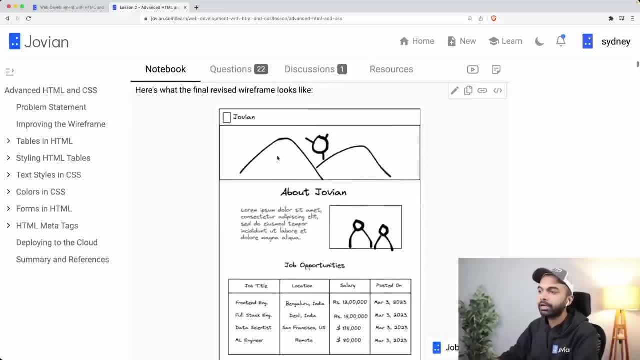 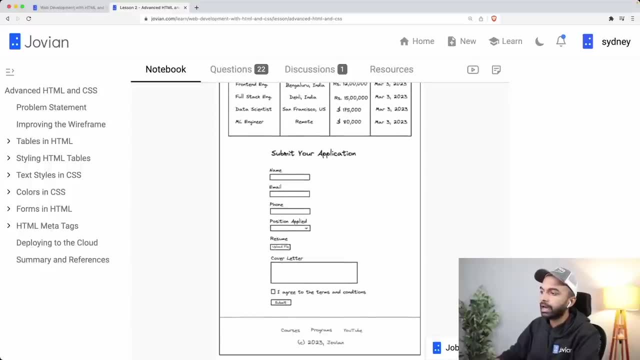 Don't do that, but just take it, live with whatever minimal content you can and just keep improving it. So here's what we decided: that we're going to add this job opportunities table, and then we are going to add a form here as well. 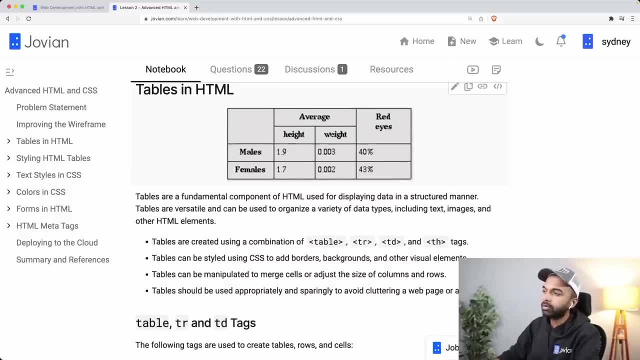 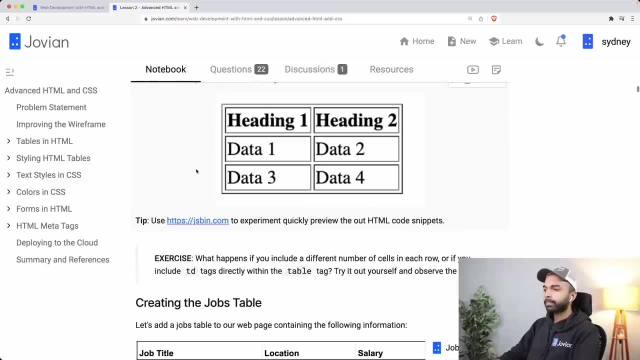 And uh, then we learn about tables in HTML and how to create complex tables like this using the table TR and TD tags. we learned about using um, the border attribute to make sure, and collapsing the border so that it looks something like that. 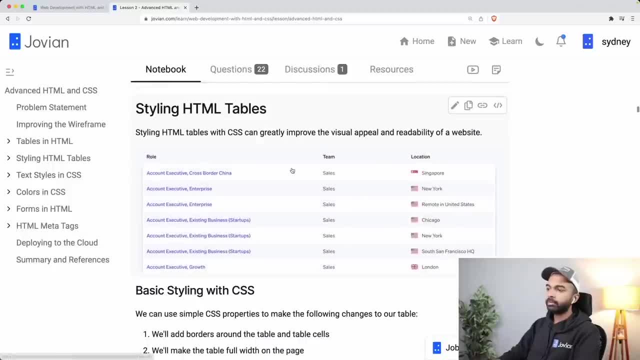 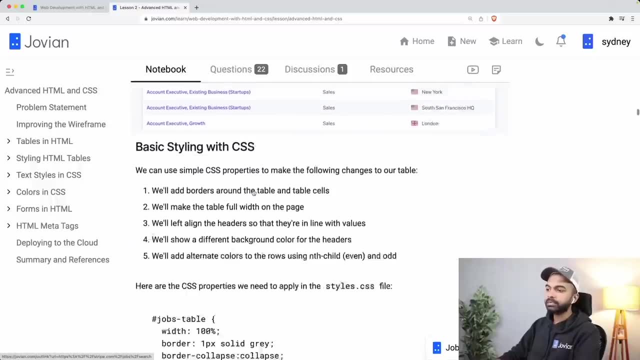 And then once we had the table, okay, So that's a table without borders. And then we saw how to style HTML tables. So again, we can add a bunch of borders, We can add a bunch of background colors, We're going to add a bunch of text styles. 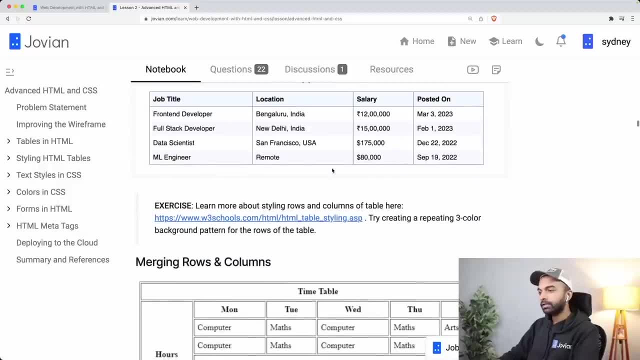 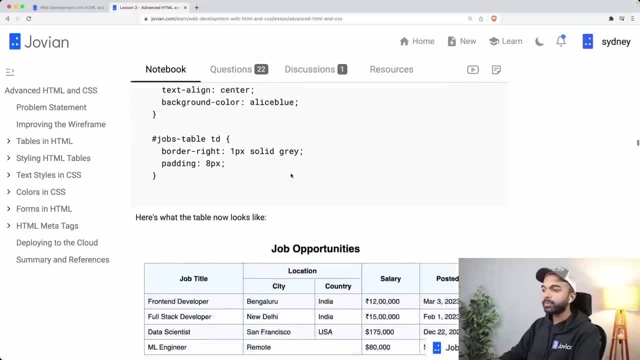 So just with a few lines of CSS, our table looked a lot better. And then we decided that we want to merge some rows and columns, make things look a little nicer. So we learned about row span, call span and things like that. 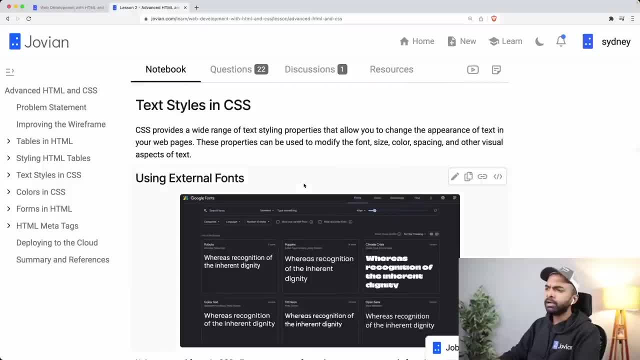 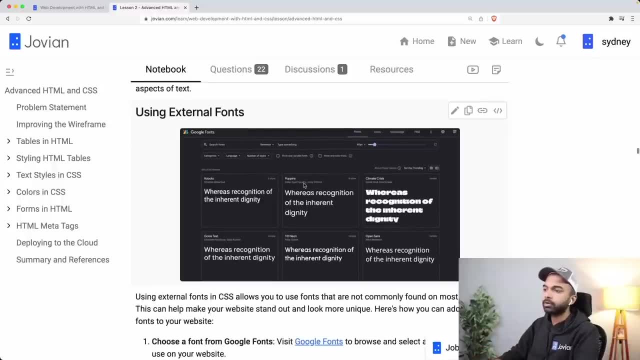 And this is what our table ultimately looked like. Then we learned about text styles and CSS. So every website, every company, has a personality, And part of that personality is the fonts they use. So to use external fonts, we use Google fonts. 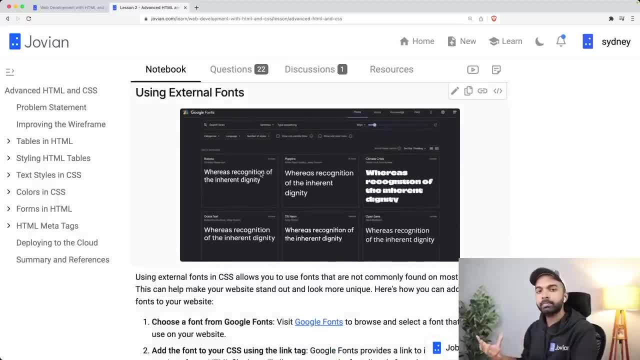 And again, I encourage you to experiment with fonts, but just pick two or maximum of three fonts: One for, maybe, headings, one for subheadings or things like that, And one for the body text. um, and make sure that those fonts pair well together. 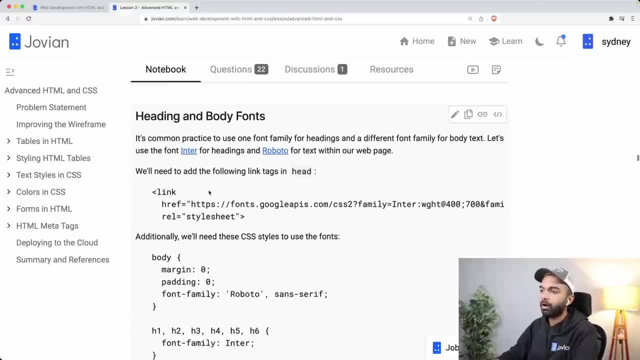 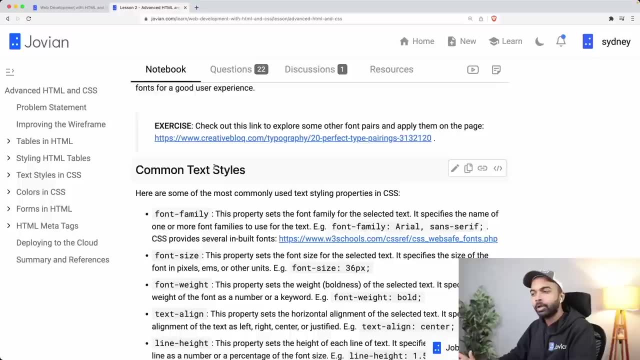 And there are a bunch of resources here that you can check out For finding good font pairings. we at Jovin we use inter and Roboto as a heading and body. uh, probably a slightly boring choice, but it does the job. um, maybe at some point we'll update that, but 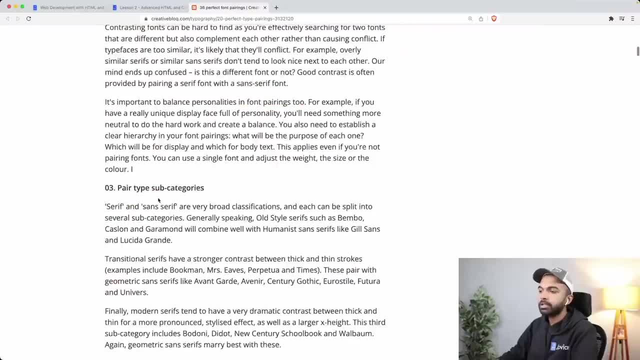 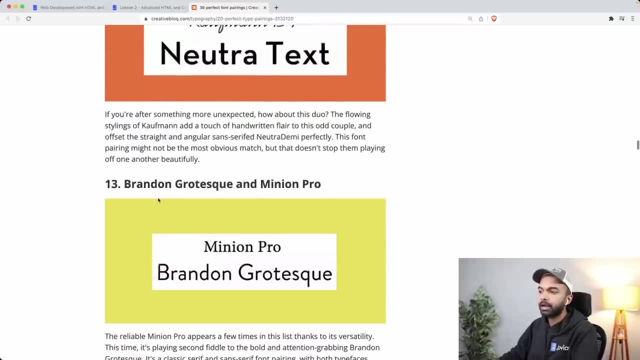 there are a bunch of pretty interesting pairings that you can check out here. Okay, So part of building your personal website is going back and reviewing all the resources that we've shared with you and figuring out something that is, um, that interests you but, at the same time, that also looks good. 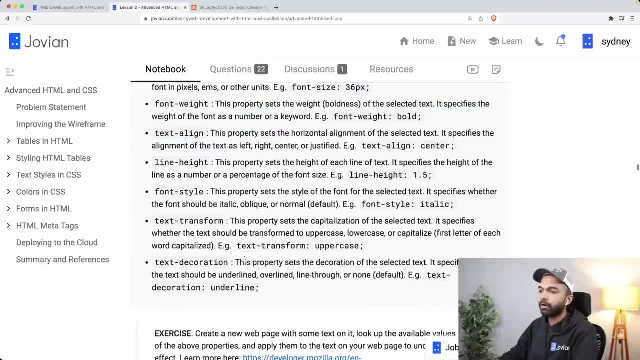 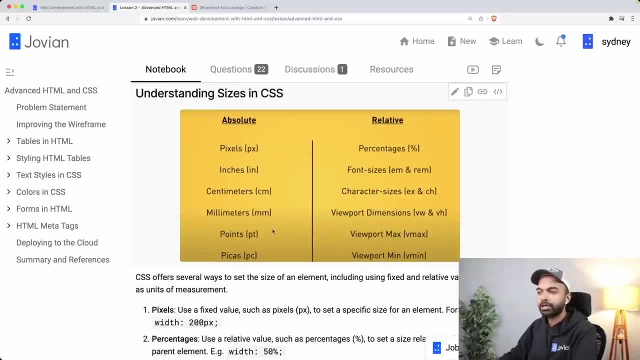 Okay, Um, so, yeah. So then, And then we learned about a bunch of font and text related properties. We learned about understanding sizes in CSS. So there are absolute sizes- Pixels are the most common, These are not really used- and the relative sizes, again percentages. 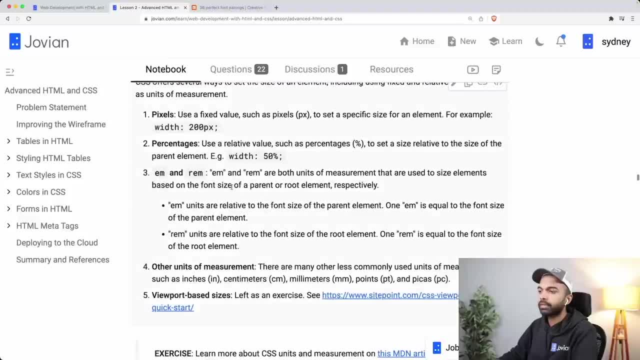 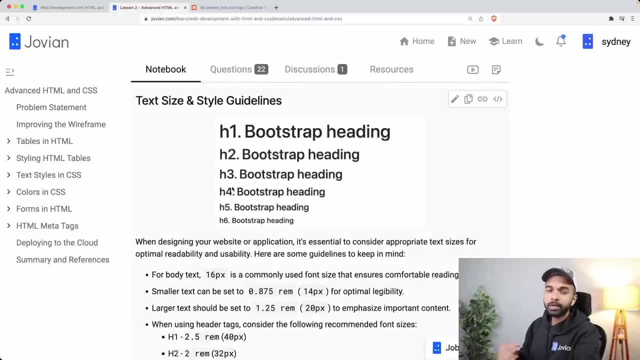 and rems are the most common. Others are not really used too commonly, but in any case you have a bunch of these sizes that you can use as well. I really want to stress again that feel free to go back and refer to specific sections. 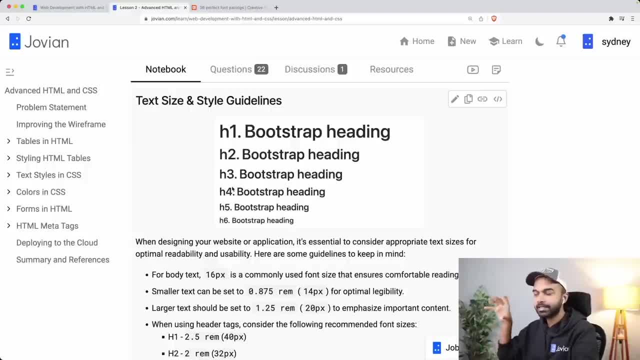 We've put, we've put in a lot into these lectures like these are things that you will keep probably referring back to for months, probably even years, as you're going through, uh, the rest of the bootcamp and also your web development, uh, uh job. 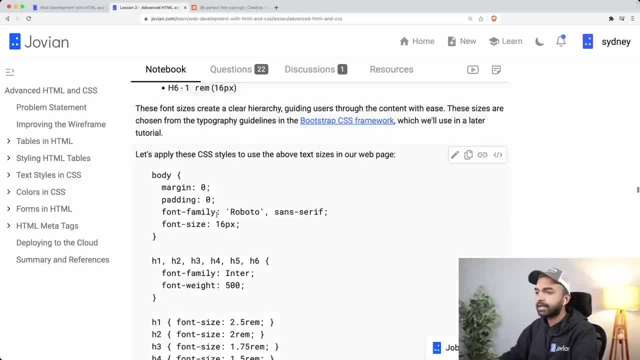 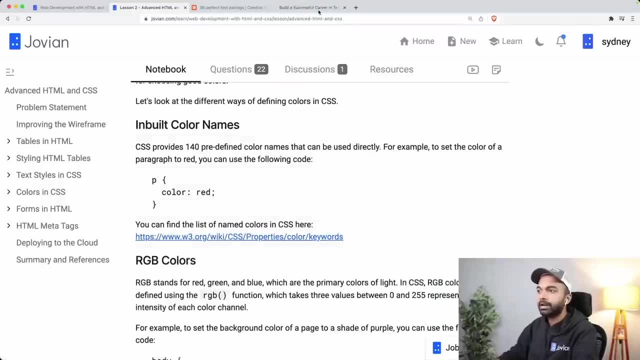 All right, Uh, okay. Then we have your tech sizes and style guidelines. Again, we have a bunch of things over here. Then we talked about colors and CSS. So there are a bunch of inbuilt colors. They are not very good for actual web design. 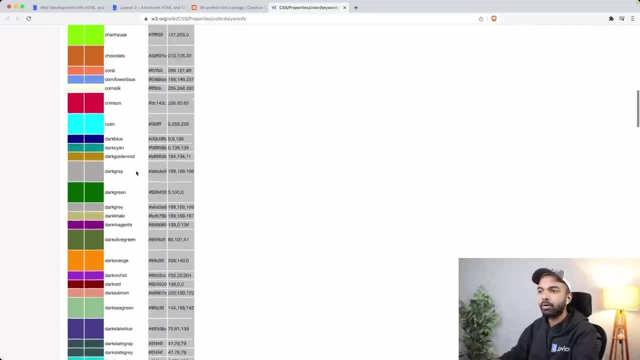 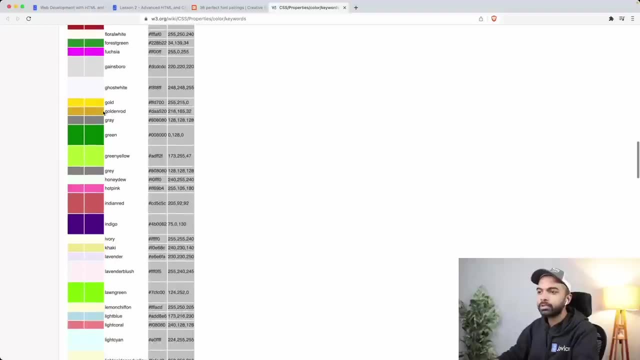 So I would not recommend using these inbuilt colors and, in general, you want to avoid something that is too bright or too Dark or too grayish. Uh, it looks very nineties. Um, you want to use something that, something that has like: um, these are. 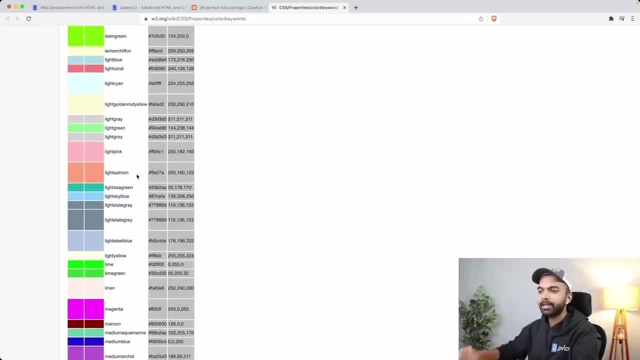 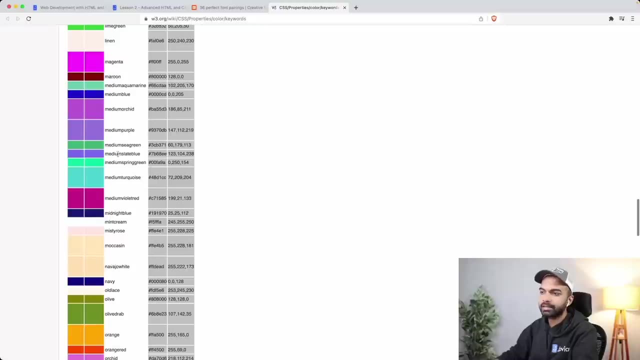 called pastels or something that is slightly dull but at the same time also has- uh, also has- an interesting shade to it, right? So these ones, uh, the uh, all of these slate green, sea green, all of these are interesting. 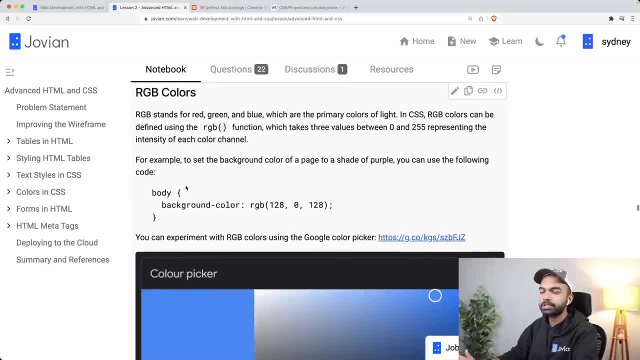 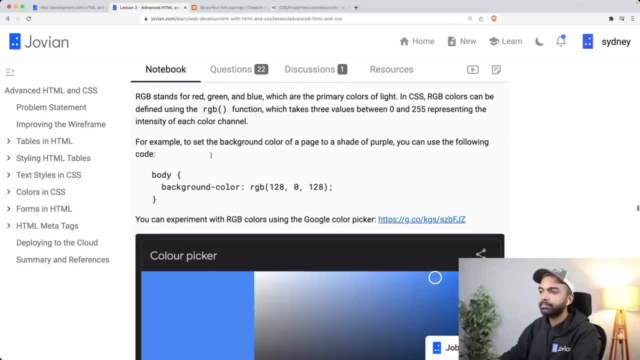 Um, but really what you should be doing is using a color palette, using some platform like a tailwind colors or something. So then we have RGB colors, So you can, of course, specify inbuilt color names. You can use RGB background, RGB values. 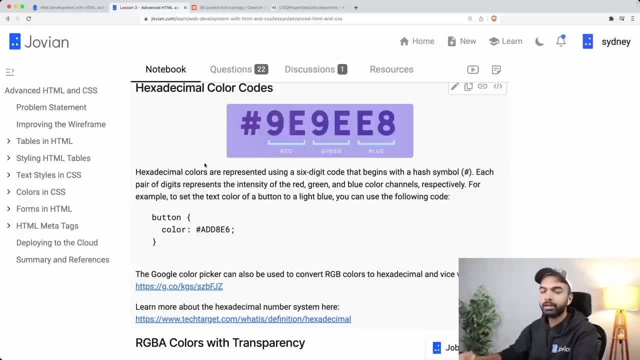 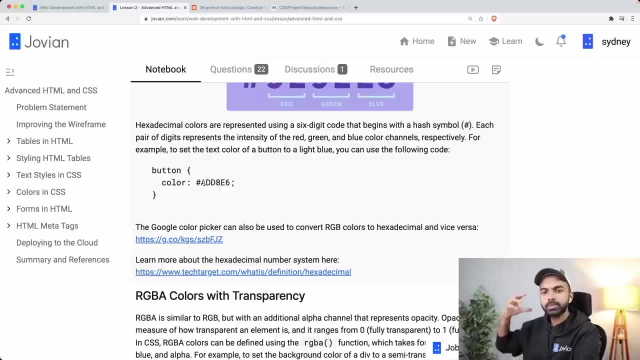 You can use hexadecimal, which is basically another another short way of writing RGB, where the first two characters represent red, the next two characters represent green and blue and it goes from zero, zero to FF. That's why it's called hexadecimal. 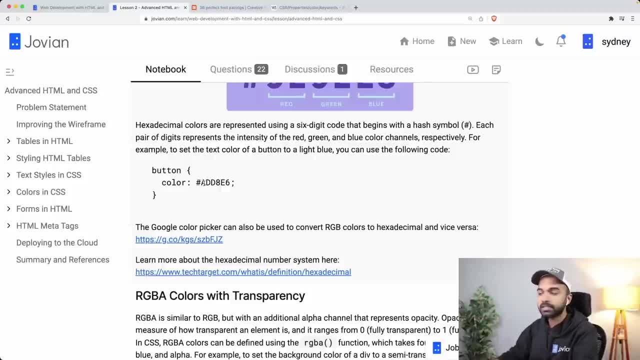 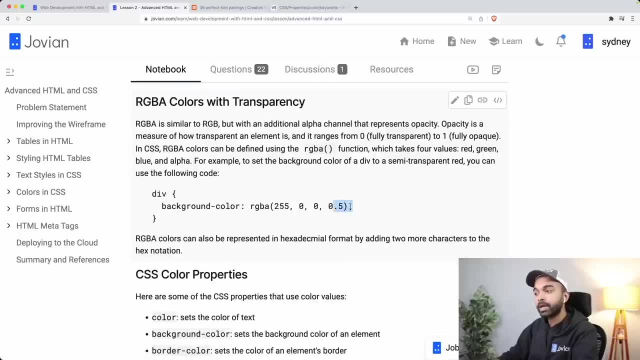 So zero to nine and eight to F? Uh, all of these are used to create numbers. Essentially, you can learn more about the hexadecimal number system If you need. you can also add transparency To your colors, whether you're using RGB or you're using hexadecimal and colors. 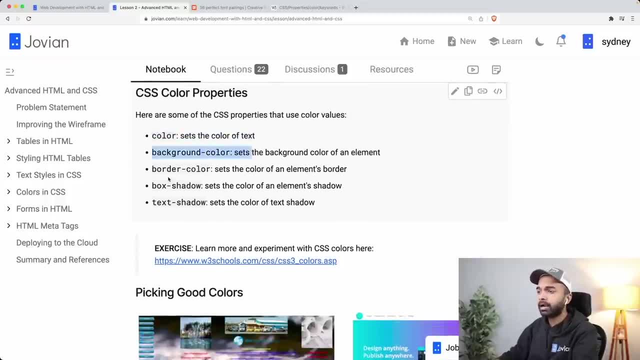 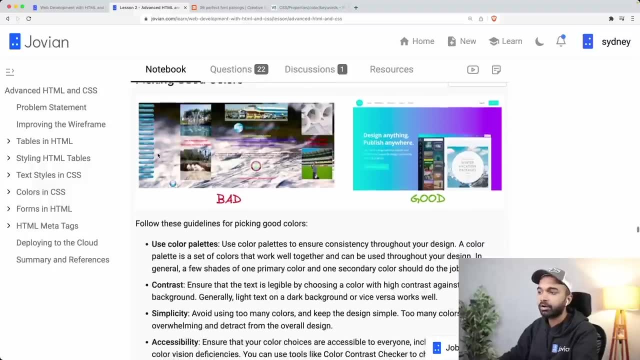 can be set for the uh. text colors can be set for the background, for the border, for the box shadow and and much more. by the way, backgrounds can also be images, So that's also something that you can check out, like this one. 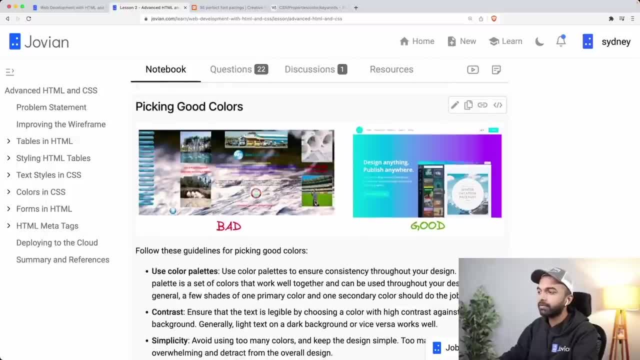 here as a background image. not a great choice, but you can see the difference between a good, consistent color scheme and fonts and a good contrast between the text and the background versus uh, a good contrast versus bad. Um, definitely your personal website shouldn't look like this. 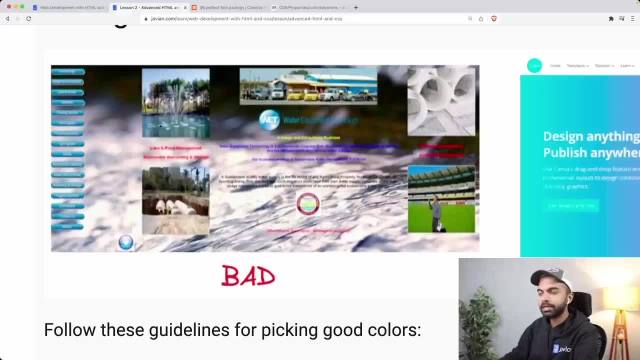 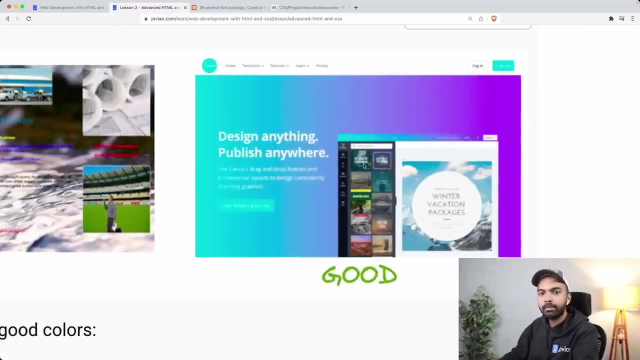 So I just want to stress here that it's very the reason a lot of the old websites look like this. uh, poorly designed websites look like this- is because this is what your website will naturally look like if you're thinking on the fly, versus if you have looked up a template, if you have decided a color. 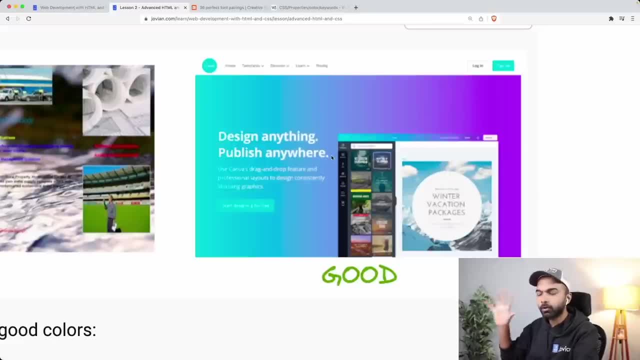 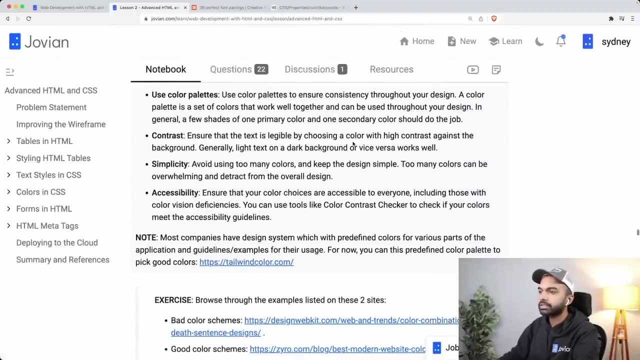 palette. if you've picked good fonts, colors, you have frozen all these details before You're actually Recording it, then your website is more likely to look like this: Okay, Um, so, yeah, so just keep that in mind. 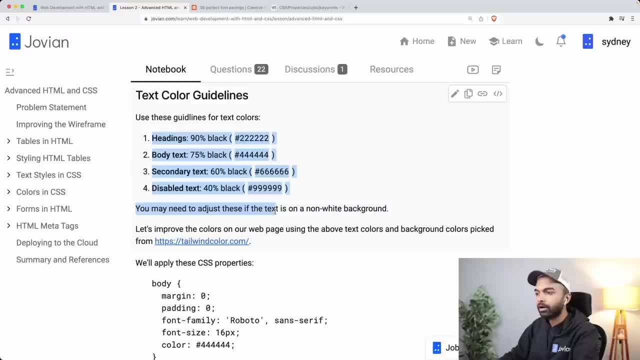 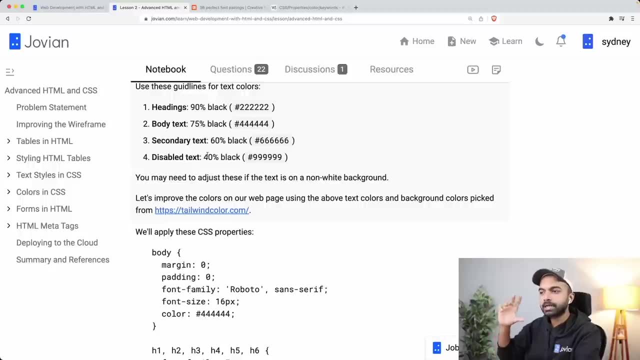 Then these are all some color text color guidelines Again. not, it's not fixed, but you can use these as a reference. So almost always you want to start out with some standard reference, something that is some somebody has figured out is a good set of selections, and then 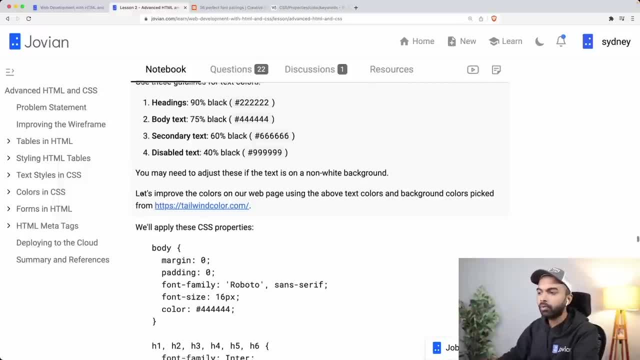 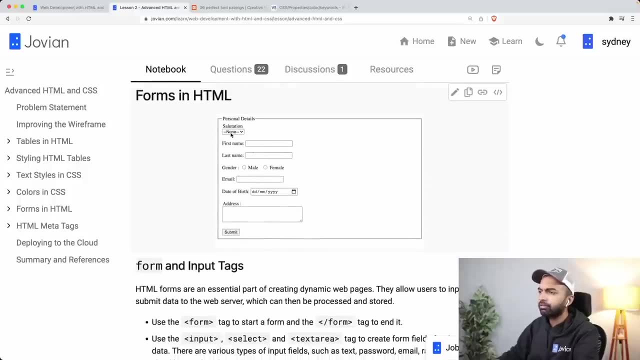 make slight tweaks to it to do what you want it to do. Um, so yeah, once we apply all these Uh, then we get back a pretty good looking site, and then we have forms as well. So forms are created using the form tag and through the input tag. select tag text. 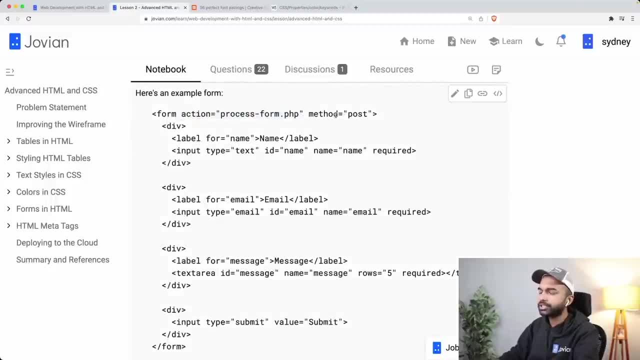 area tag and we also use the label tag. So every form has an action And again, this could be an external website, This could be maybe a server endpoint you have implemented and a method, but you create divs and inside the divs you create these labels and you have a bunch of 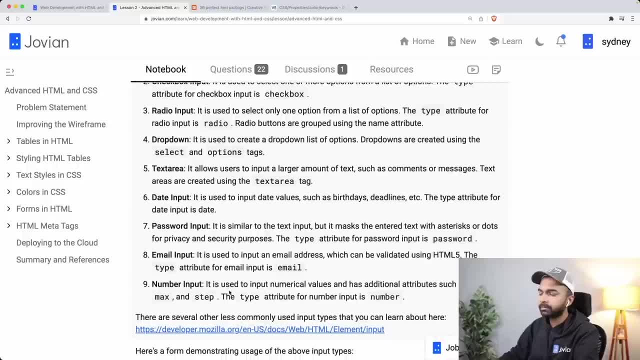 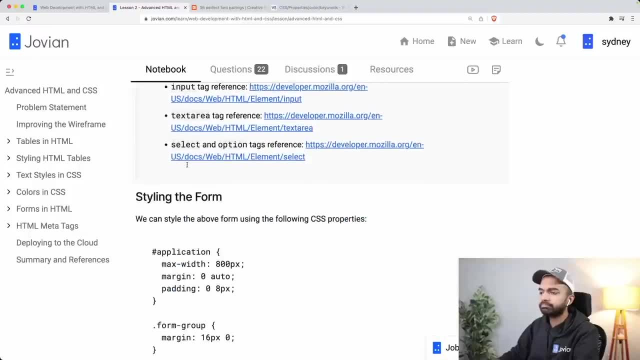 different types of inputs: text, checkbox, radio, dropdown, Text area, password, email, et cetera. And once you've put in a form, then, um, you can style it. You can give it a bunch of different styles, and this is what a form. 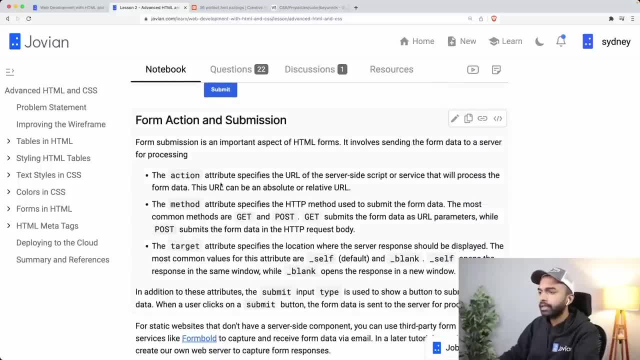 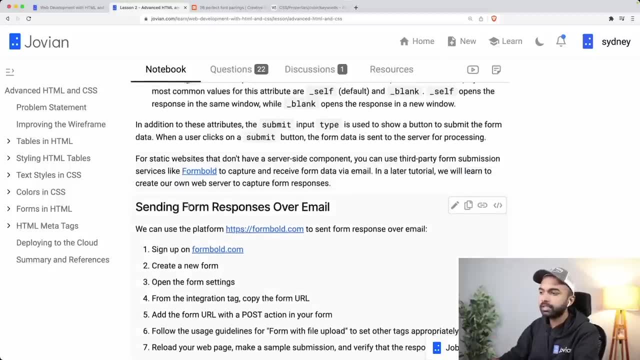 might potentially look like: Okay, And then there's an action and a method and a target. So in this case, well, uh, we used form board because we were not talking about servers early on, So you can just use any service that can receive form responses. 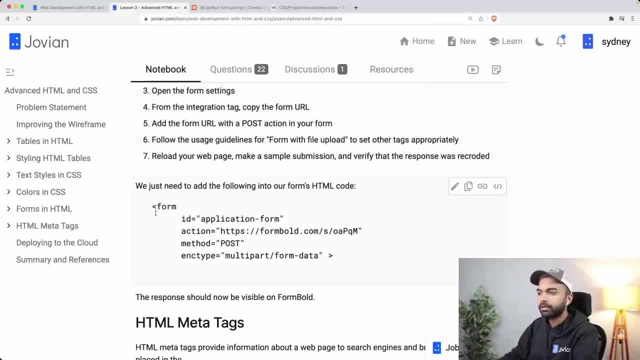 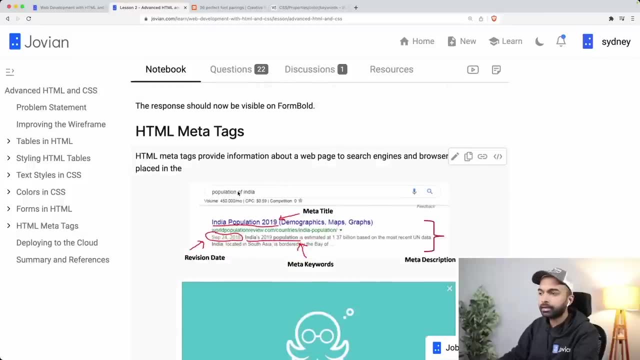 Form world is a good one, Useful one, uh, in case you don't have the option For the time to set up a proper server, and we simply pass it's action method, et cetera, and it can collect whatever we needed to collect. 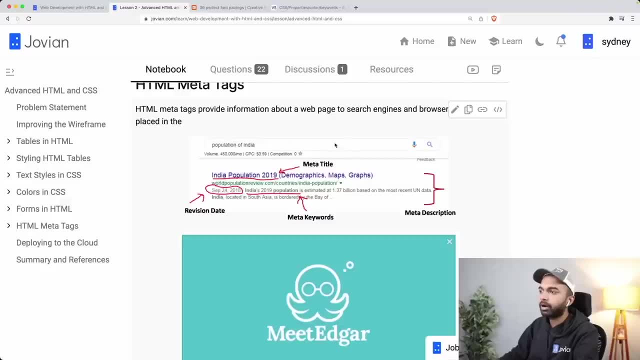 And then we have, uh, HTML meta tags. meta tags provide information about our webpage to search engines and browsers. So when your website is searched online and Google finds it and shows it in a search result, that is when all these meta tags will come into picture. 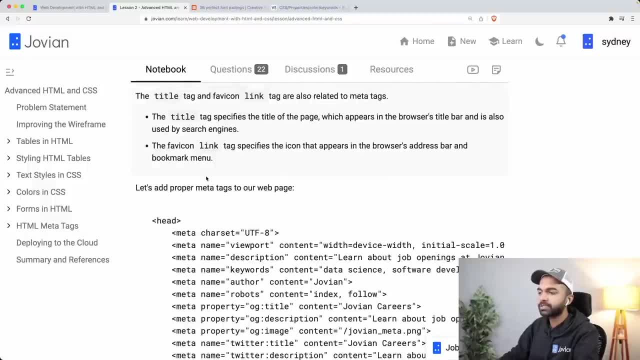 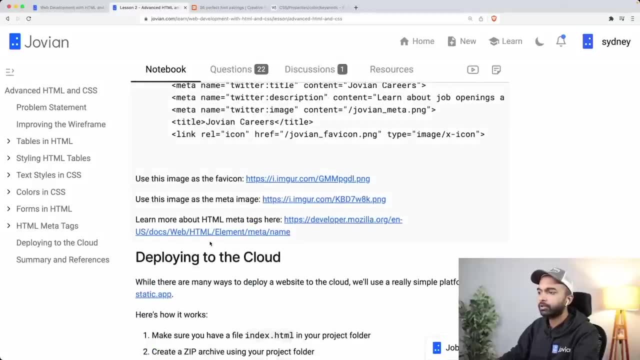 Okay, So these are some common meta tags and these are some platform specific meta tags, and then there's a title and favicon tag that are used to change the browser title And favicon. So that's again something that you can um set up as well, right? 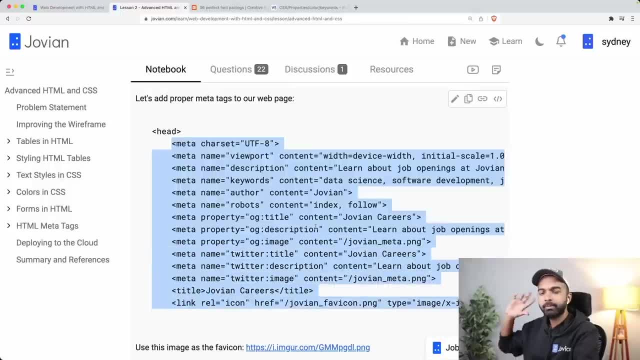 So you should, you can literally just take this set of meta tags, paste it into any website that you're building. I think one requirement we should, we will add in the project, is that it should have, your website should have proper meta tags, um so that it can. 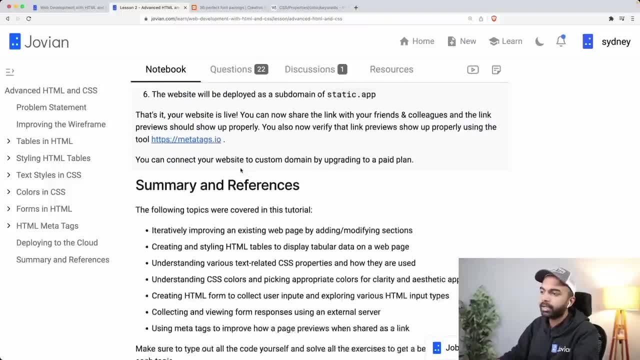 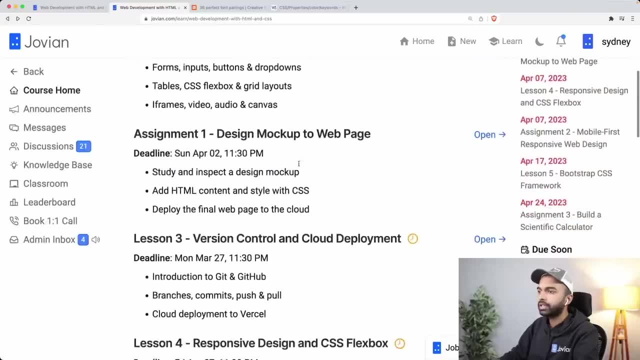 be shared easily by with other people as well. and then cloud deployment. Again, we were still talking about, uh, static app here, because we are not touched on gate and GitHub. So that was lesson two. And then you had an assignment where you had to convert a design mock-up into a web. 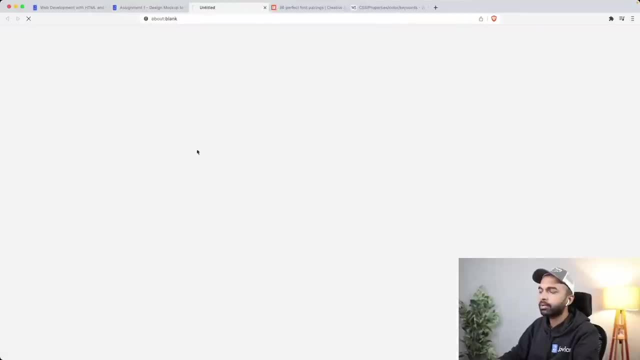 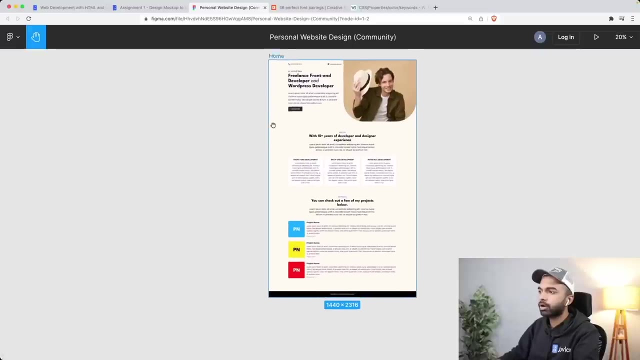 page. So you had this design mock-up and what you did was you had to inspect it using Figma and to set up a basic page structure and styles. This is the mock-up over here You have to set up the basic page structure and styles. 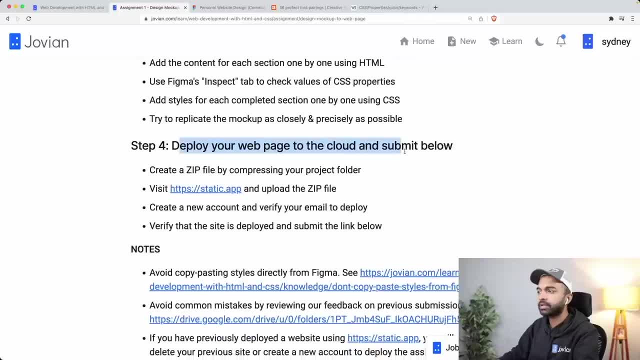 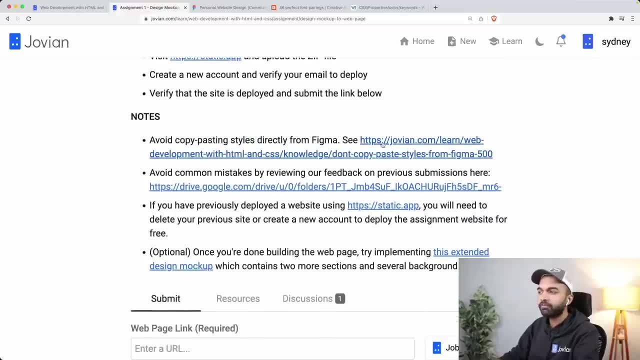 Then you have to implement the webpage section by section. Then you have to deploy your webpage to the cloud and make a submission Right. Um a few tips: avoid copy pasting styles directly from Figma. So there's a knowledge base article on this, and we've also picked up a bunch. 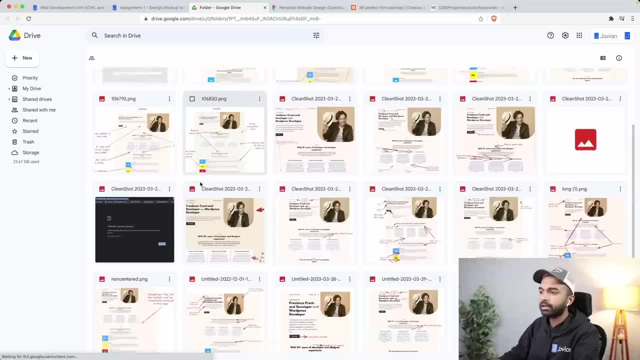 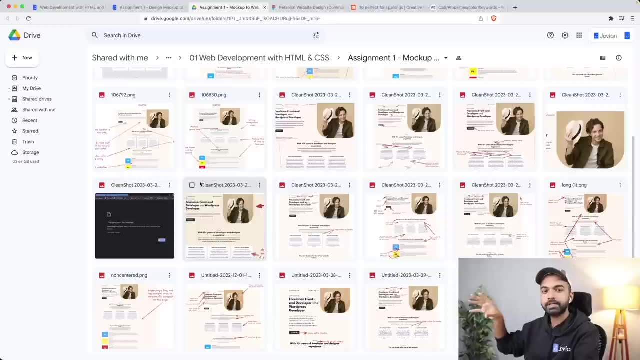 of common mistakes and put them into this Google drive folder. So again, use these, go back and refer to all of these for your personal website as well. Your goal should be to get a pass grade on your first submission, And for you to get a pass grade on your first submission, make sure that. 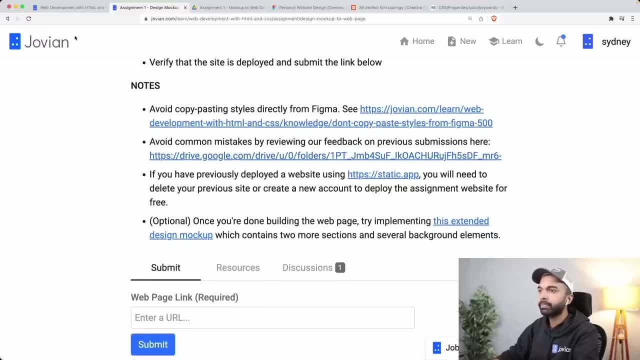 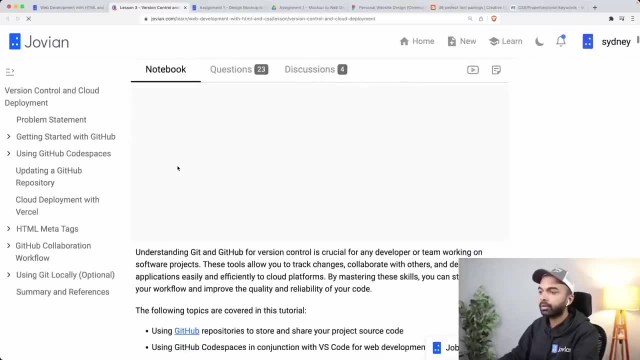 you're not repeating the mistakes that you or other people have made. Okay, Um, that was this first assignment. Then we talked about version control and cloud deployment- the proper, uh way to do web development- And that is where we talked about Git and GitHub. 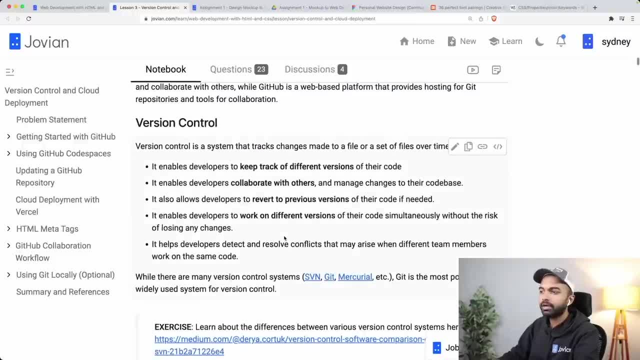 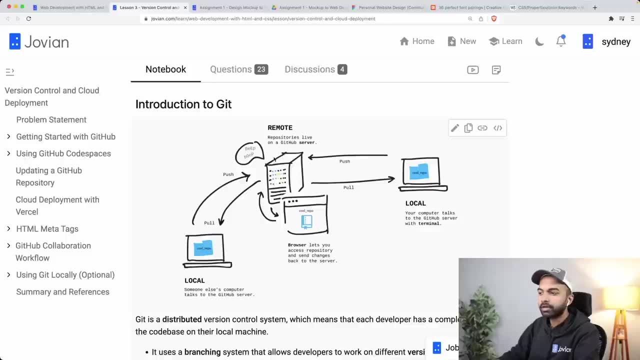 So we started by just getting started with GitHub Uh. we learned about what version control is, how it is useful. We learned about Git uh, where you basically you put your code on a remote server and then you can pull it into any computer or maybe a cloud computer like. 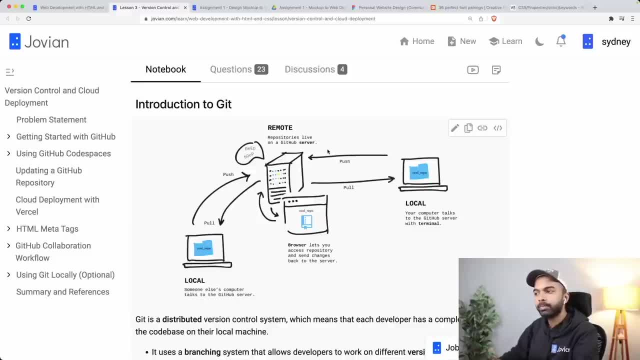 GitHub code spaces and you can make some changes and then you can push it back and still have all the older versions available, And you can also view it from the browser on githubcom, And you can also Collaborate with other people, right. 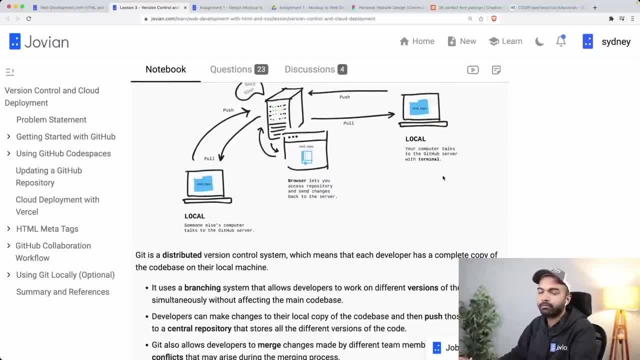 So again, there's a lot. Git itself is a huge thing that for years, people um keep learning or just try to manage through, uh, just running a few simple commands. That's what I do. I just remember three or four commands and use them all the time and look. 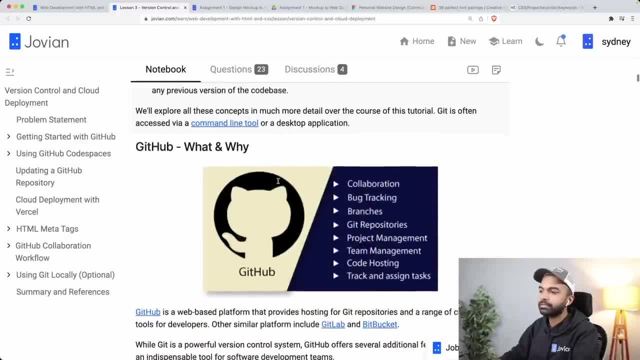 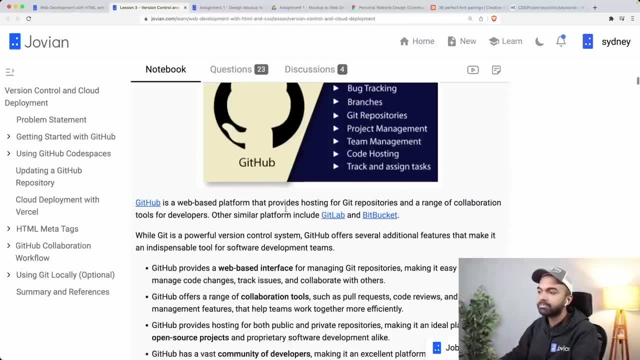 things up whenever I require, but this is a basic structure of what Git gives you, And GitHub gives you a bunch of abilities on top of uh Git. It is basically a web-based platform that also gives you some collaboration tools. uh, it's where you can find open source projects. 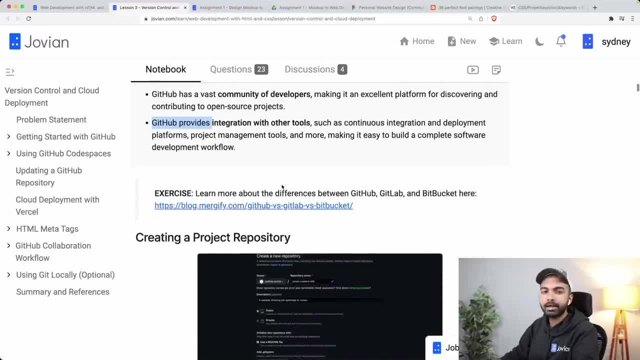 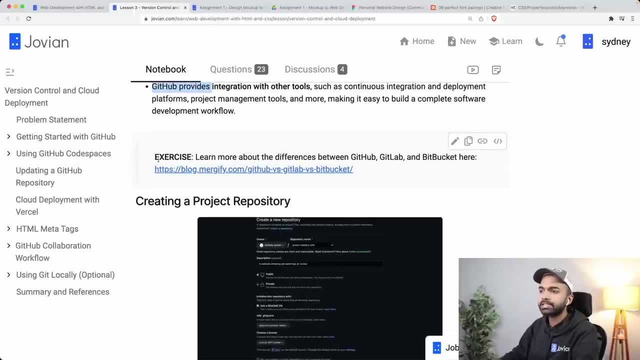 It has a wide community and it has great integration with other tools. I didn't, And for uh web developer, that GitHub profile is kind of like the resume, So we'll talk at some point about actually creating your own GitHub. uh, read me a profile as well. 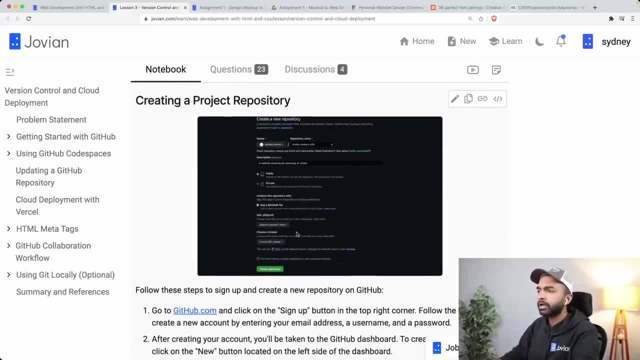 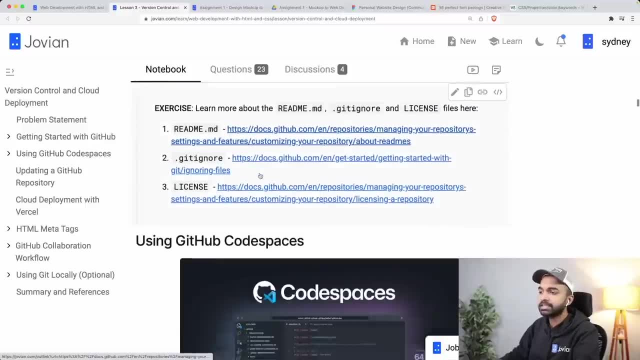 Okay, We'll cover that at some point. So here, yeah, we talked about how to create a project repository, and then you have these things called a read me and a get ignore. We talked about them as well- And a license as well, especially if you're building an open source project. 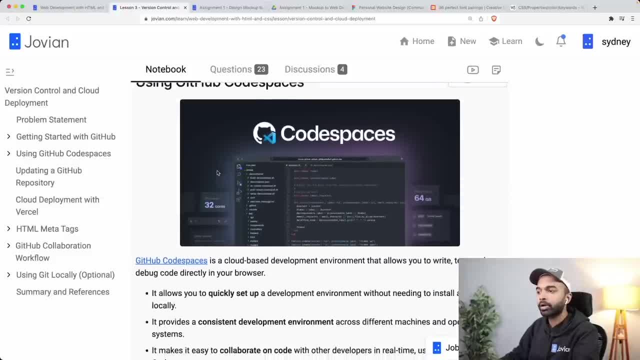 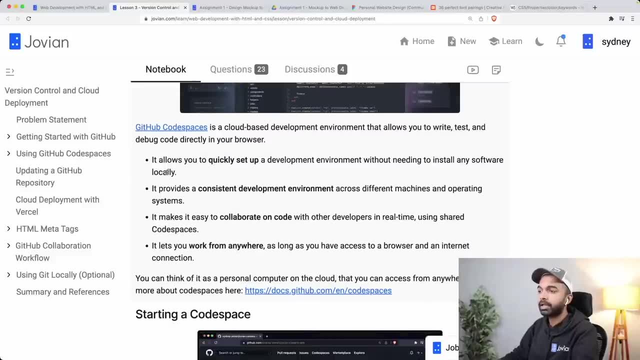 And once a project repository is created, we talked about how you can open it up using GitHub code spaces, a cloud-based development environment with a free tier that allows you to write, test and debug code directly in your browser. Quick to set up, gives you a consistent environment. 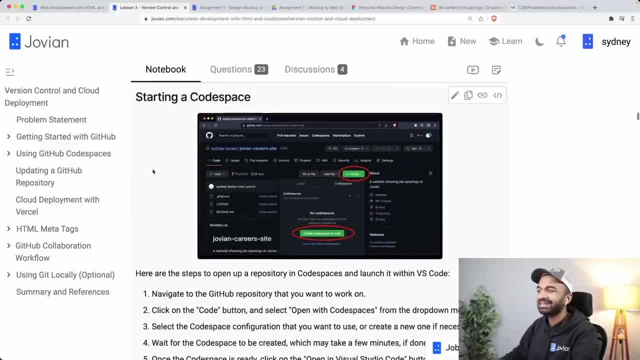 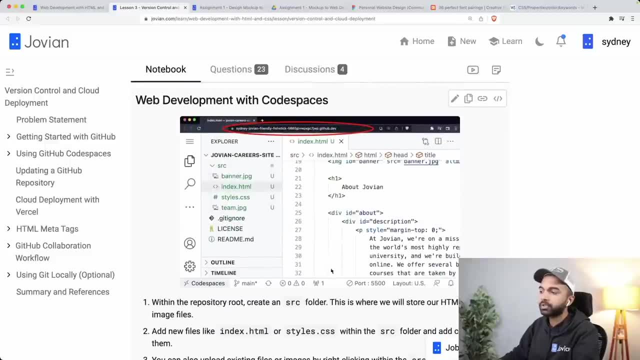 You don't have to install anything, Let's you work from anywhere. and starting a code base is really easy. You just click the code button and click create code space, and that's how you can create a code space, And it gives you this visual studio code interface in the browser, which, honestly, is good enough. 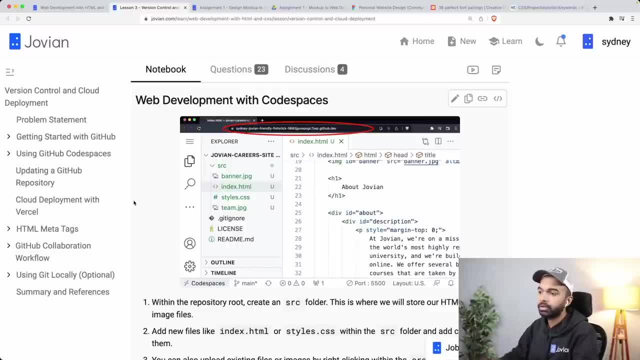 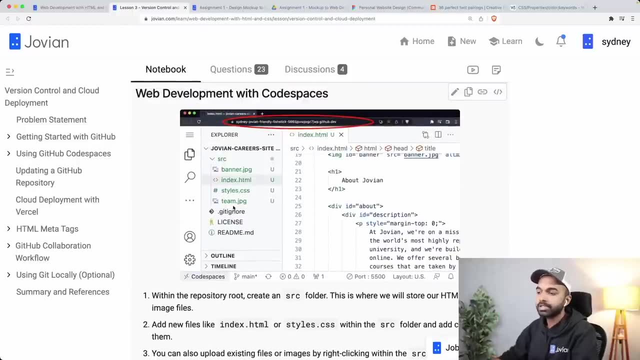 That's what I've been using for a bunch Of projects that I've been working on, and you don't even need to install anything on your computer and you can install extensions within this VS code browser and they will remain there the next time you try to open it. 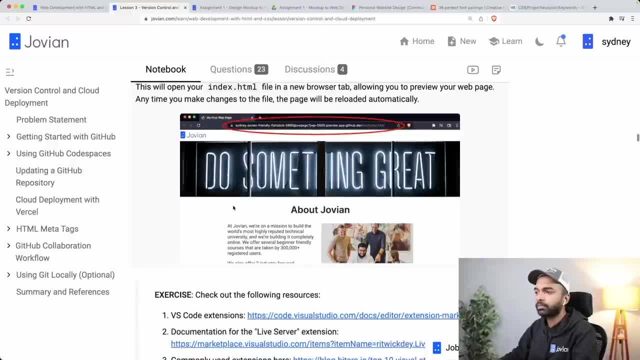 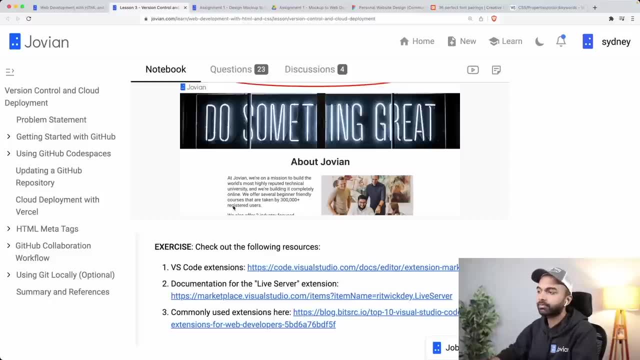 So we at Jovian have almost all completely shifted to get up code spaces. We still do use our local machines because the free tier is not sufficient for some of our work. That's why, Um, yeah, and then you can run it using a live server. 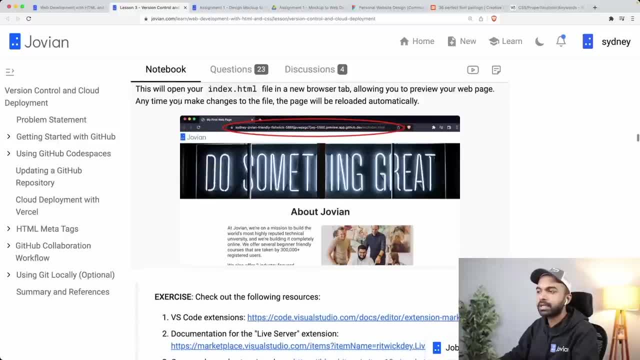 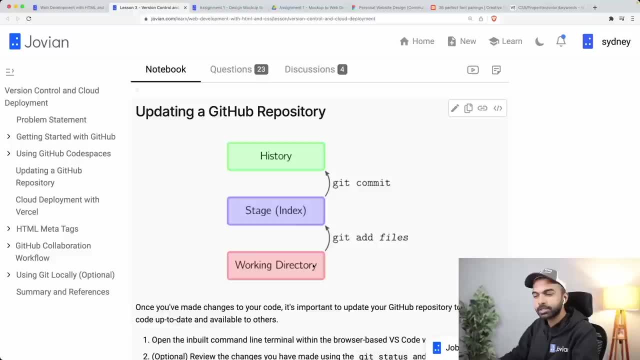 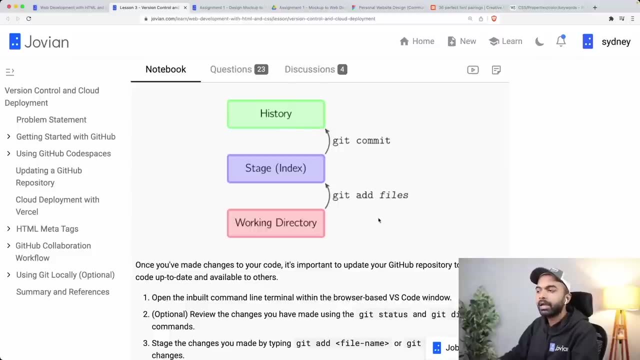 So, especially when you're developing a simple HTML and CSS webpage, you can Just use a live server to run things and then get a updating and get a repository. It's fairly straightforward. It's a three-step process, but there are buttons to do it in one step. but you just first add files and stage them and then you commit them and then you push them. 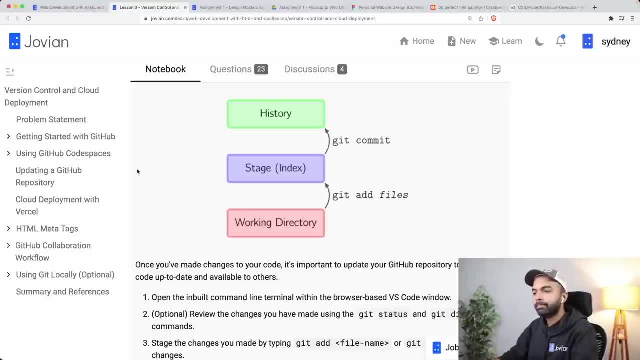 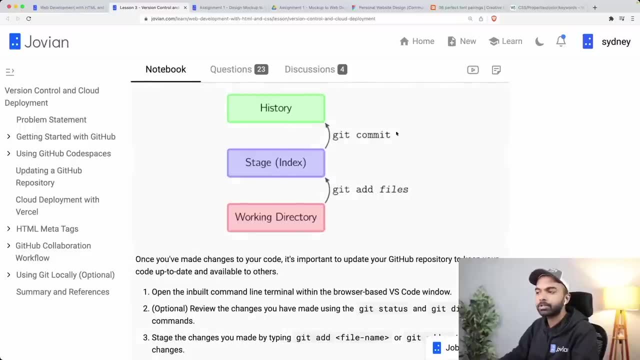 Right, So each of them has a certain purpose, a reason they were built, Um, but what you should just remember is that all these stages are important for your code to actually reach the GitHub cloud repository. All right, So make sure that you are always going to add push. 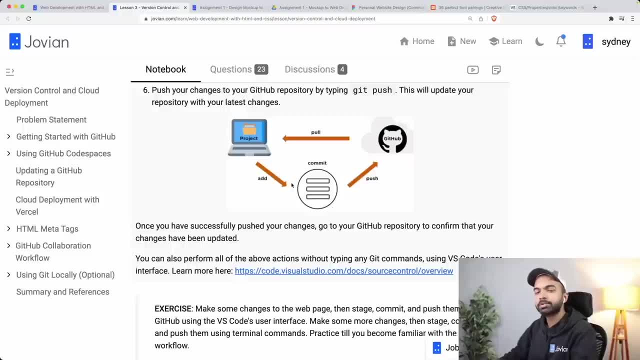 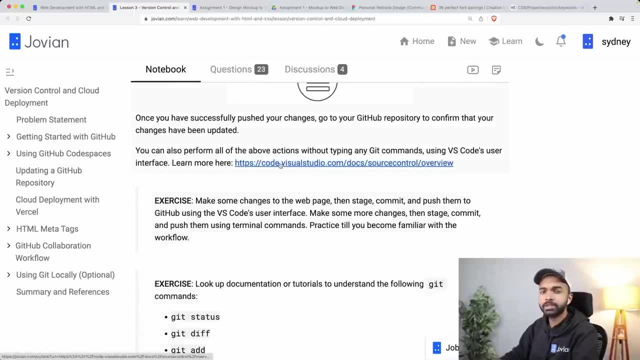 And then add, commit and then push. So add is going to stage your changes, Commit is going to record a new version and push is going to push it to GitHub and then somebody else can pull it. And there are ways to just do this using a visual studio code, so that you don't have to run anything on your end. 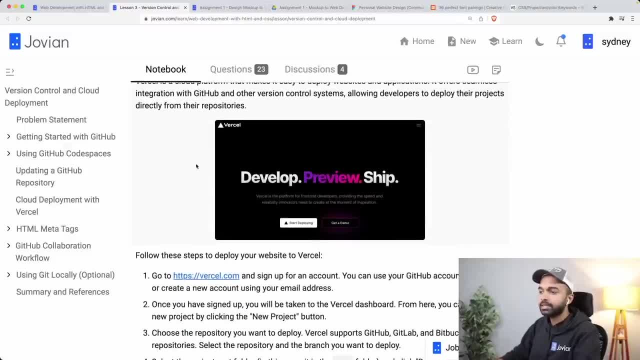 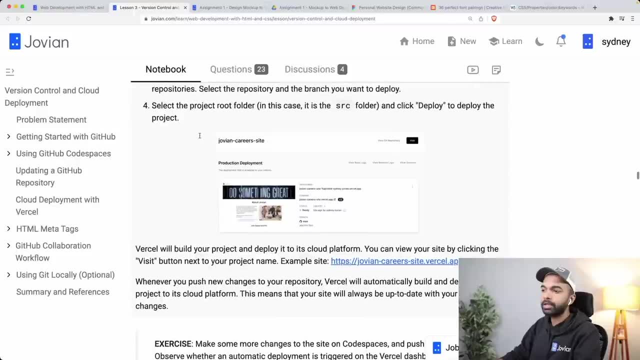 Then cloud deployment with Vercel was again a breeze. All you do is sign up on Vercelcom and you connect your GitHub account. Then you select the repository that you want to deploy and you select the folder inside which your actual code is present. 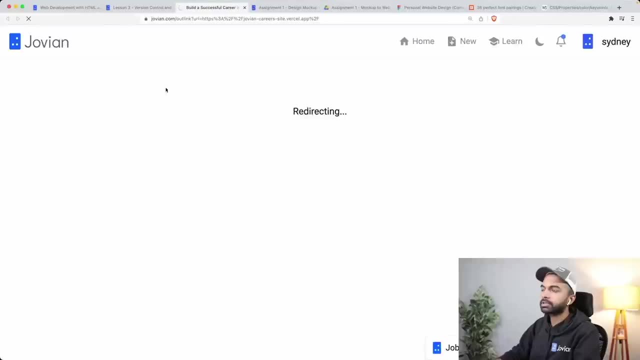 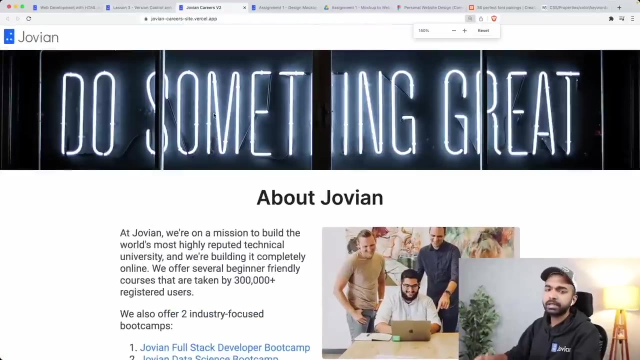 That, um, that Needs to be deployed, and it's going to deploy it for you, And it's going to look something like this: So this was actually the website that we deployed and, um, yeah, that still looks fine And it's going to be there. 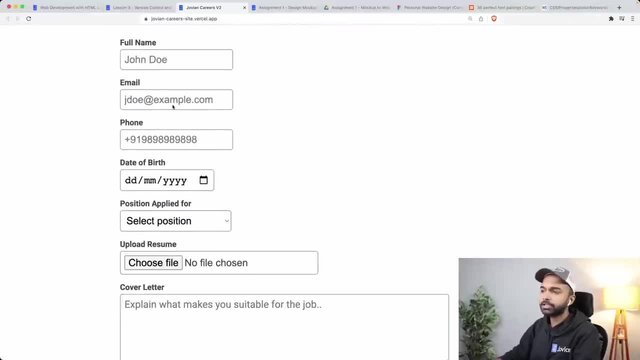 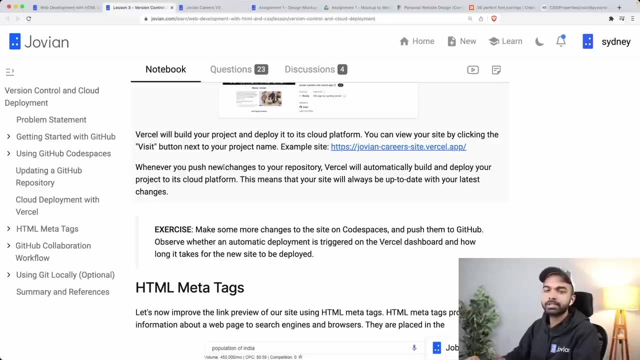 So you're going to have all these old versions of your websites, or uh, for each repository. Vercel is free. It has a good uh, huge uh, basically an unlimited free tier, unless you start hitting significant amounts of traffic, at which point it will make sense for you to pay anyway. 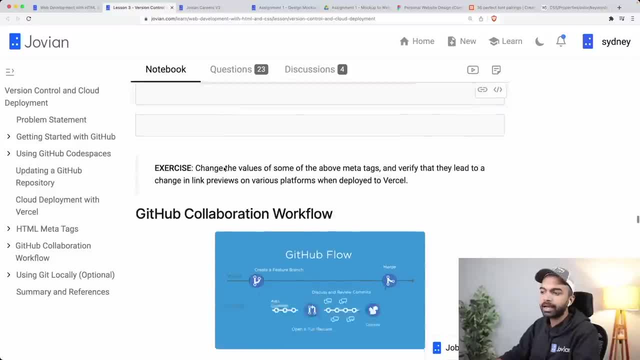 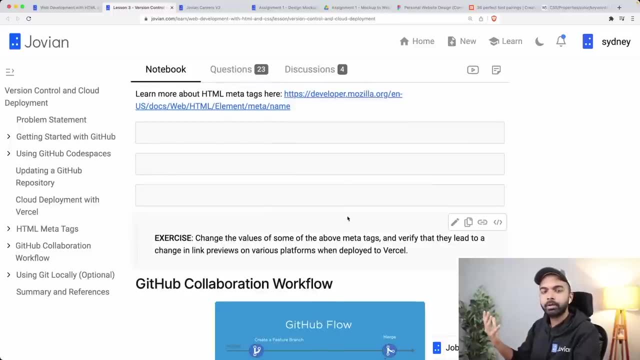 And finally, once again, we just covered tag, talked about meta tags. So meta Tags are pretty important because you want to be able to share your work with other people And when you share it it's kind of the cover for your book. 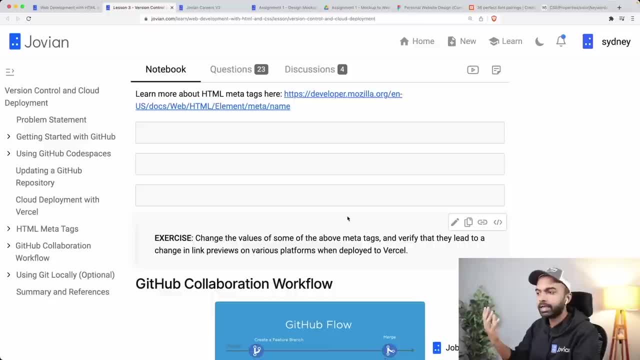 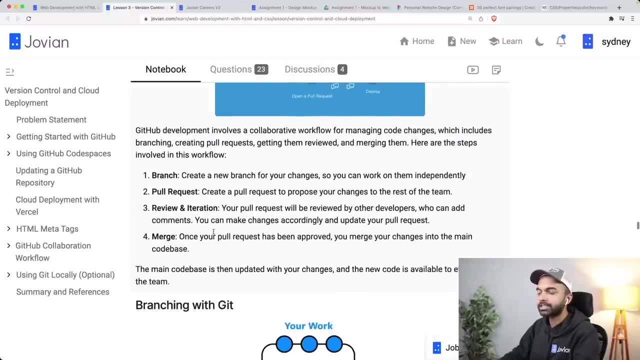 Uh, if the website is your, if your website is the book, then the meta tags, which is a meta title and image, are the cover, and books are judged by the cover. So, similarly, websites are judged by their meta tags. All right, 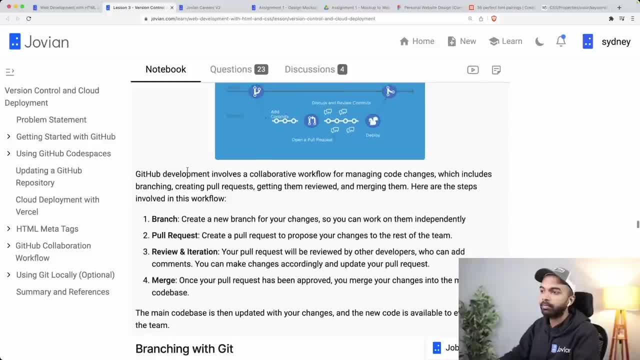 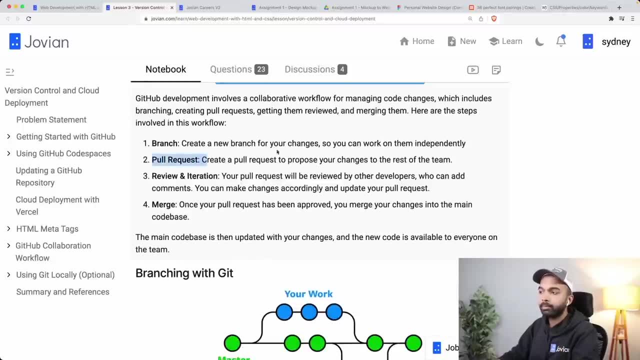 And then the we talked about the GitHub collaboration workflow. when multiple people are working on a repository, the way you should work is create a branch. Then you should create a- uh, make it Changes on the branch by making a bunch of commits like that. 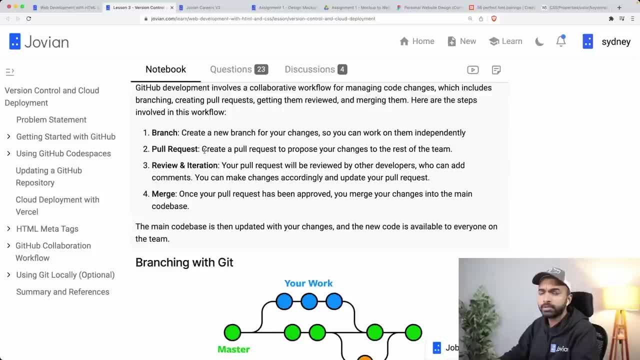 Then you should create a pull request where somebody from your team can, or even just you yourself can, review the changes And then you can, based on the comments you can make, uh, you can update your branch and keep pushing more changes And finally you can just merge, uh the merger branch to the main branch. 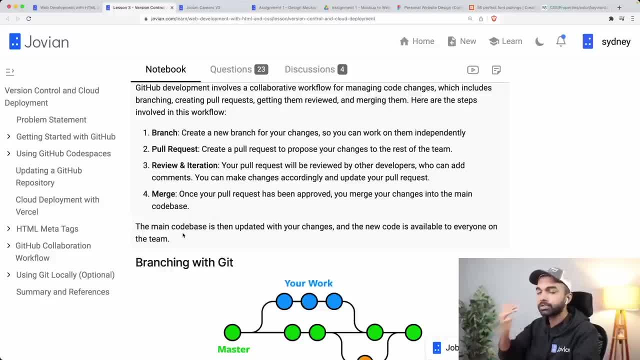 And just like that, your changes will then get deployed automatically If you're using a deployment platform like Vercel, right? So whenever you're doing any new development and this you should try to apply to your website, Uh, uh, website. 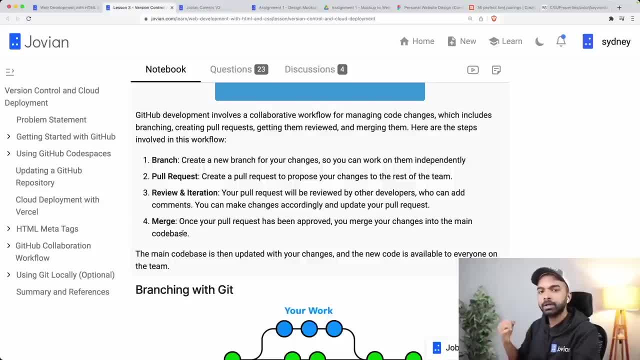 As well. once you've pushed out the first version, then for the second version, make sure that you create a branch and then you keep pushing your changes into a branch and keep updating a pull request, And when you've done enough work that you feel it's ready to again go live, then push it back. 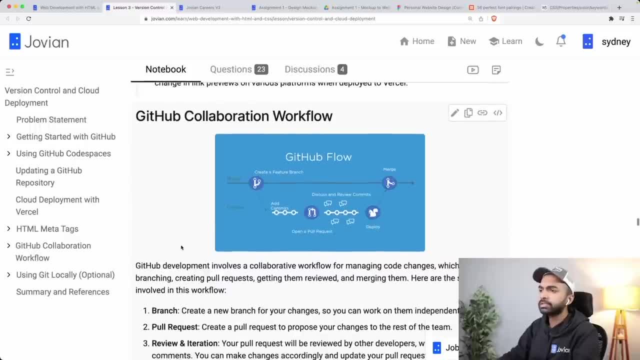 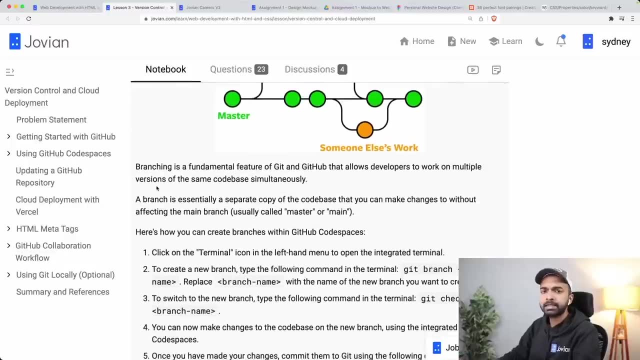 Okay, So Try, practice, uh, practice using the GitHub workflow here, the GitHub flow for your work, Um, it's also again just good practice And it's something that you can talk about when you are, um, let's say, when you're sitting in an interview. you can mention. 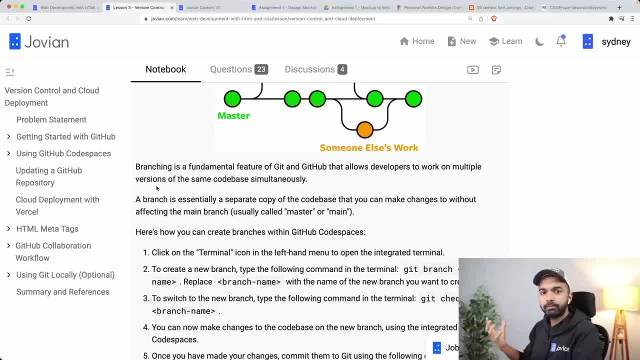 I mentioned that when I built my personal website, I used the GitHub flow. So first I created a simple uh page with just my picture and a few lines about me, and then I deployed it to a cell and then I created a new branch. 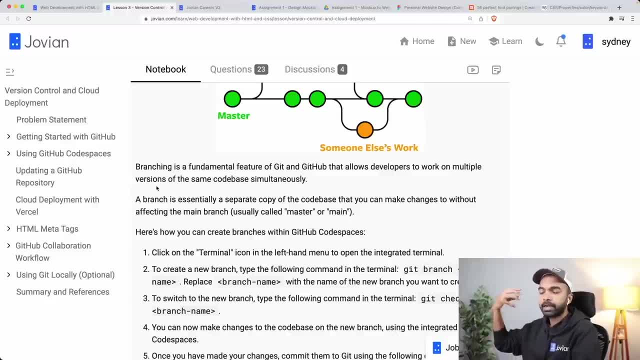 And on that branch I added a project section, I um created a pull request, I tested it, I reviewed my own code and only then I merged it back. And then I updated, and I did that three, four more times to add multiple things to my website. 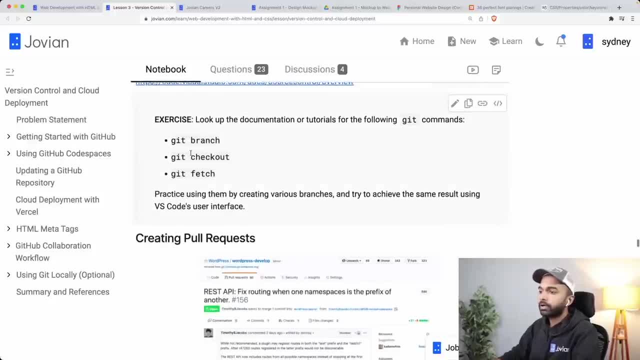 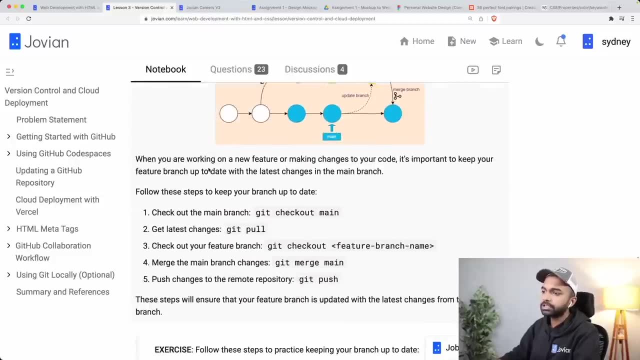 Okay, So try to do that, Try to follow the GitHub flow for sure, And it'll help you. Then creating pull requests. Well, pull requests are uh. again, there's a flow here. then keeping a branch up to date. 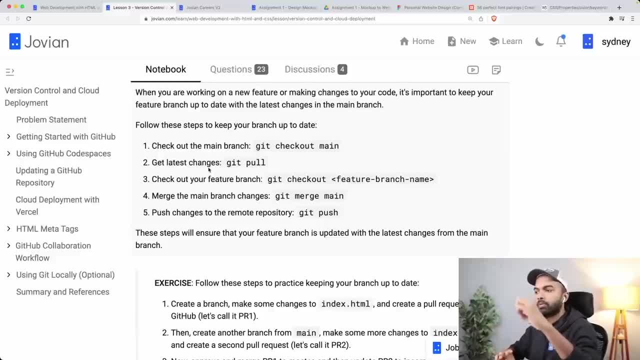 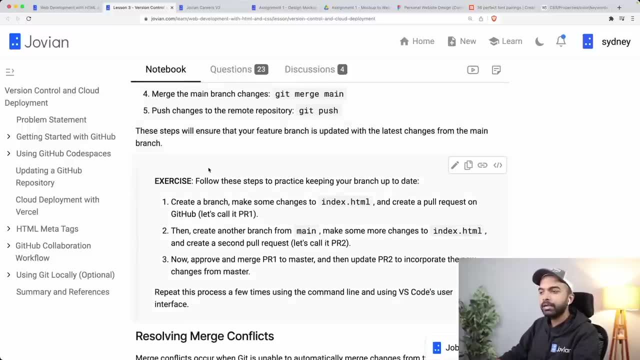 So sometimes the master branch and the main branch will go forward, So you'll have to pull those changes back into your branch and all that. This makes more sense when you are working in a team- whether actually other people working in as well- and you might run into merge conflicts. 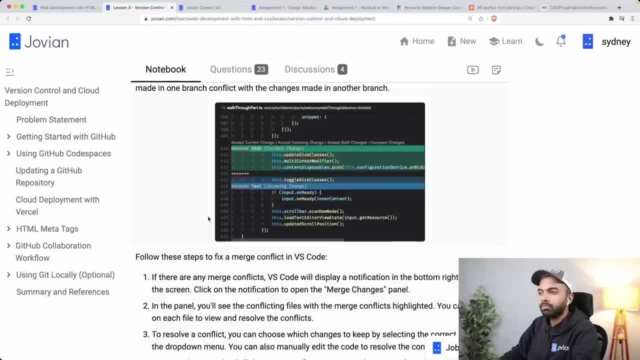 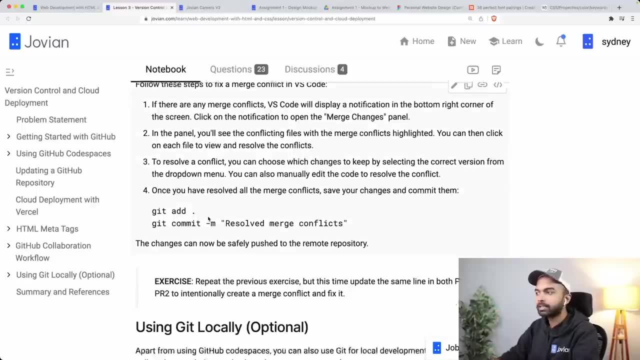 You might have to fix them. Uh, not something that you have to know by heart, or not something that you will be doing on a daily basis, but you can always come back whenever you want to review this topic, So there are a bunch of resources here that you can check out. 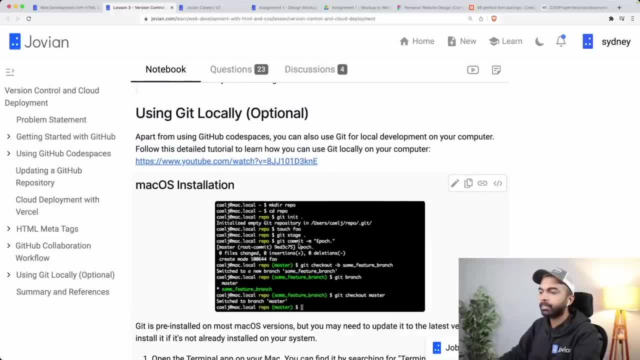 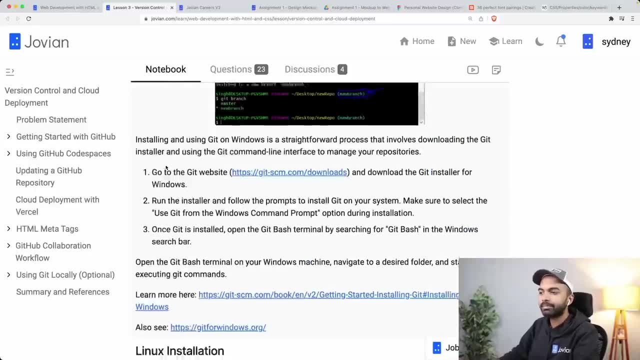 Okay, Regarding merge conflicts and regarding, uh branching, of course get can also be installed locally. So if you're up for it- not a challenge exactly- but if you want to put in the work to actually set up get locally, you can go ahead and do it. 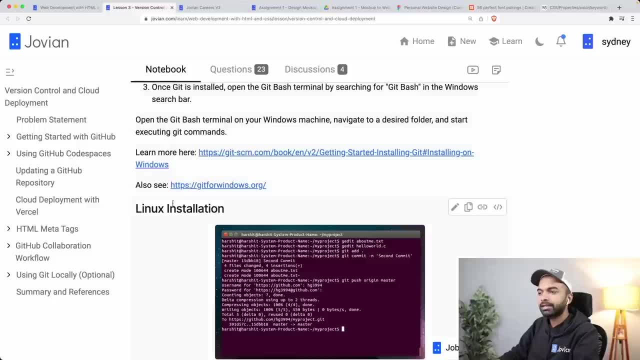 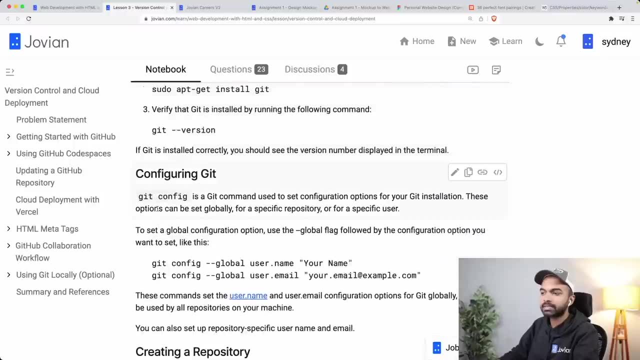 I wouldn't say that this is a necessary anymore, because either your company will be using something like GitHub code spaces or they will give you a laptop with all of these things pre-installed, So I wouldn't worry too much about it, Okay. 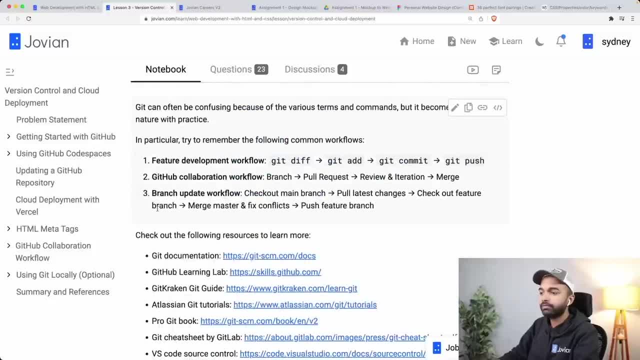 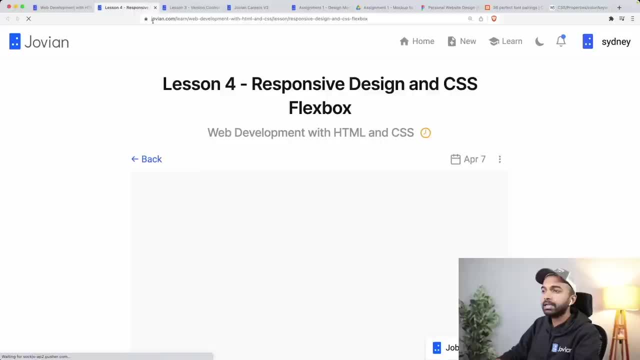 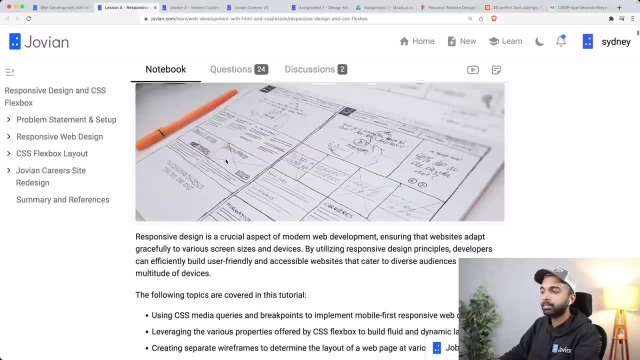 But all the information is here and you can always look it up whenever you need to, So feel free to come back to all of this whenever you need to look into it. Then we talked about responsive design and flex box. So this is now we got to a point where we want to make our websites look good not just on our desktop development screen, but also on mobile screens. 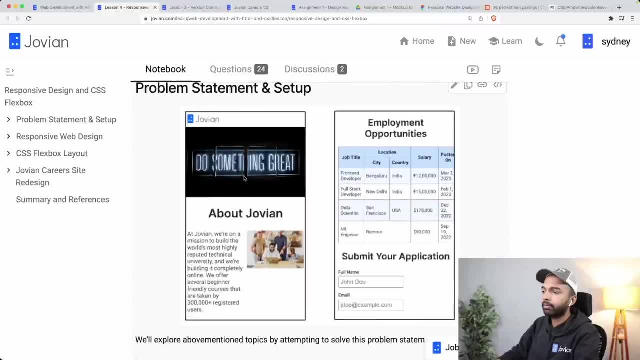 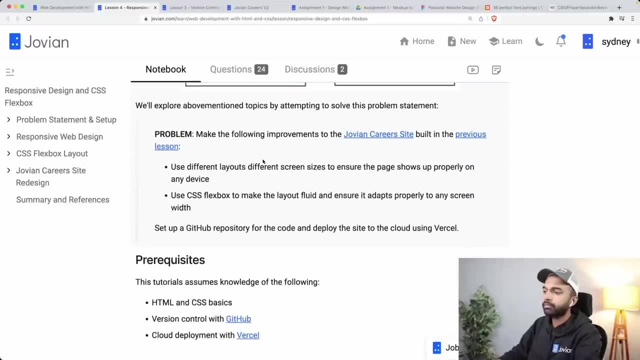 So this is where, uh, we wanted to create um. so we saw that the website that we had created doesn't really look very good on mobile and we wanted to create the website and we want to make it more responsive and to do that. 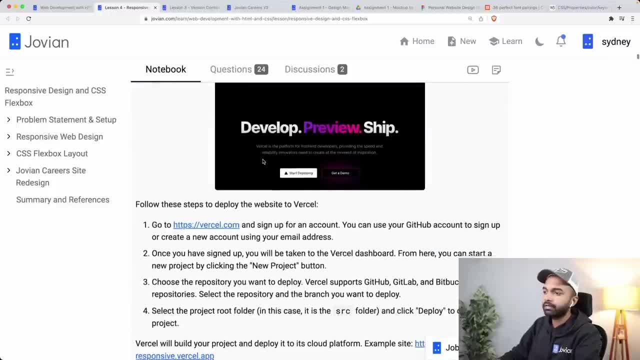 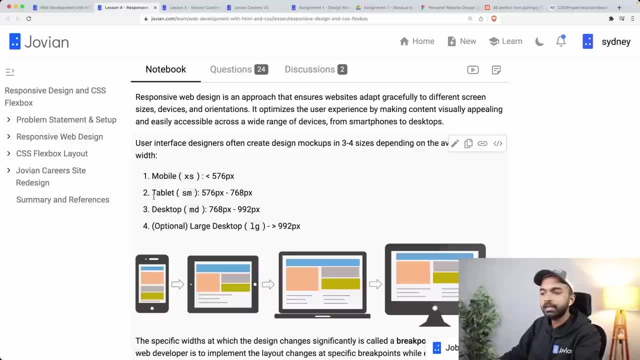 Well, first we duplicated the GitHub repository that we had and then we deployed it once again, open it on GitHub code spaces, And we learned that for responsive design we have to break up our design into three, or maybe at least two, but maybe three or four, uh- different designs. 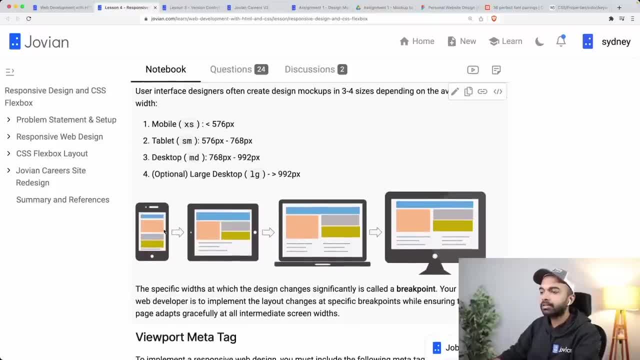 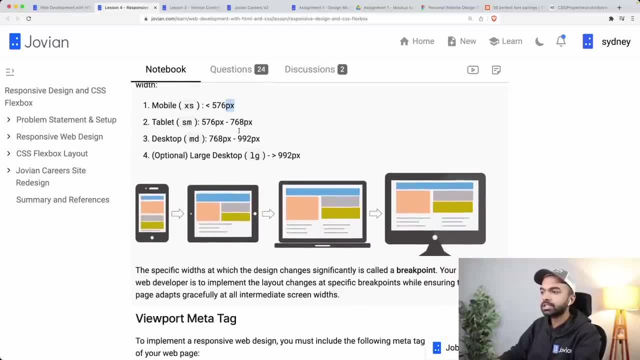 And at each break point, which is at each device with, the layout will change a little bit. So here you can see that at now, for small screens, the layout looks like this and then suddenly, at about five, 76. pixels, the layout is going to shift into this. 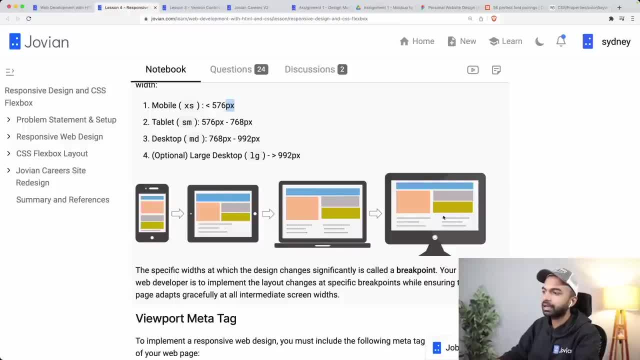 And then the last layer is going to shift into this: at seven, 68.. And at nine, 92 is going to shift into something else, right? So this is a very common pattern. Almost all websites follow it. at any websites made in the last 10 years, 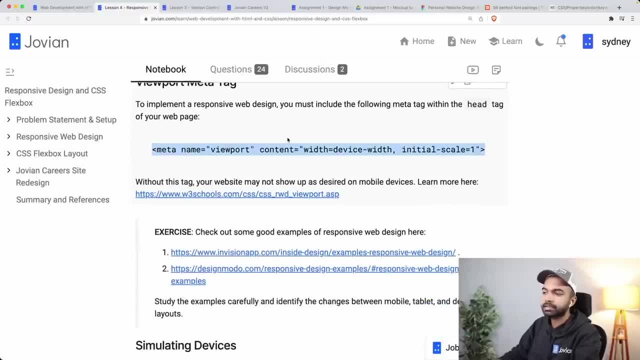 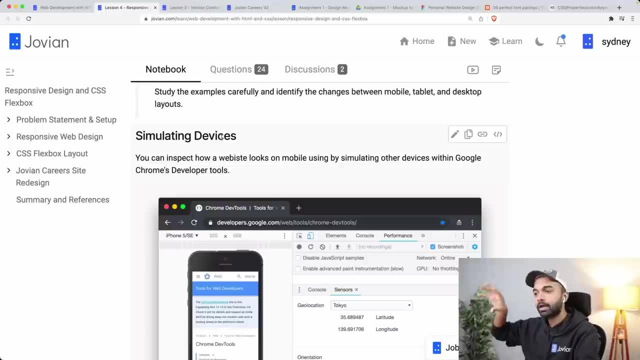 We'll. we'll follow it. I do enable it, though You need this meta tag. This is often something that is forgotten, So make sure you do that again. A lot of these instructions are not necessarily given on the project page, but you'd have to go back and see how to make these happen. 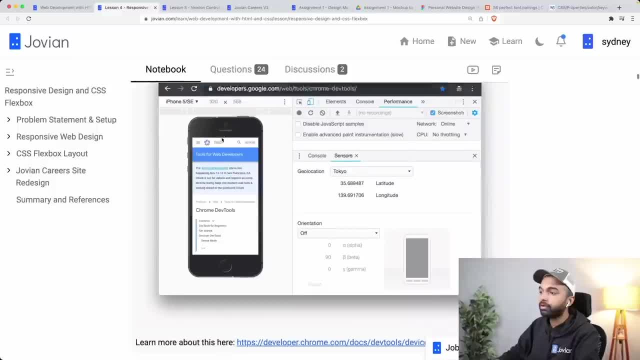 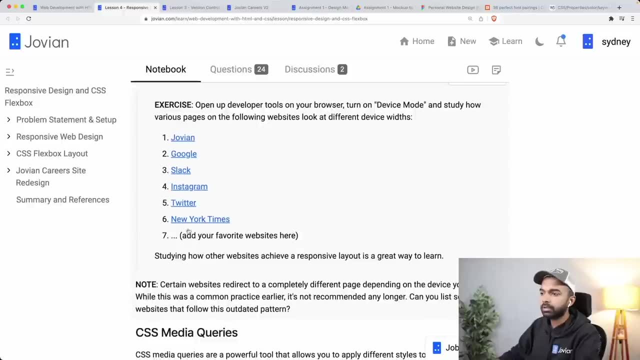 Okay, So it's also a way for you to review all the content. You have More on your browser, using which you can test the response or the response or layout of a website, And you can create a way to just see how other websites are achieving. 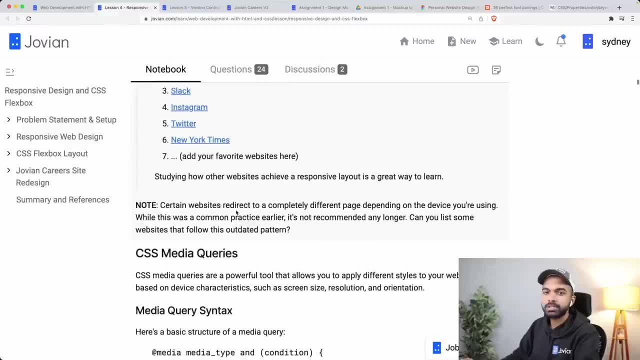 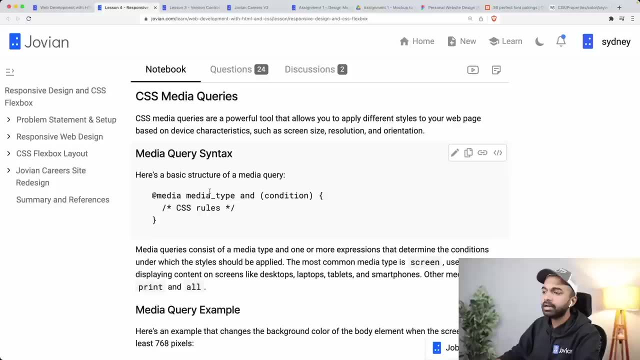 Responsive design is to just open them up on device more and see what they do. Now the way responsive design is implemented is using CSS media queries where you can provide at media you can product media type and a condition And when the condition is met, for example, if you say min width seven, 68.. 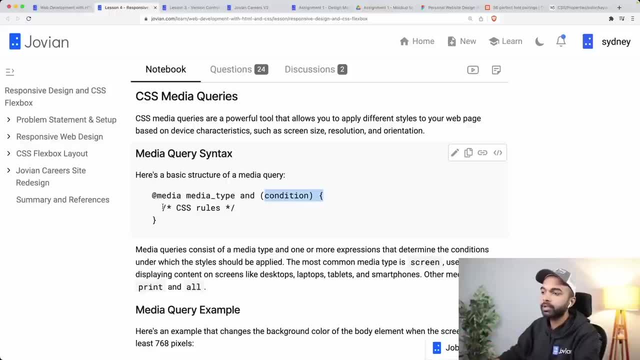 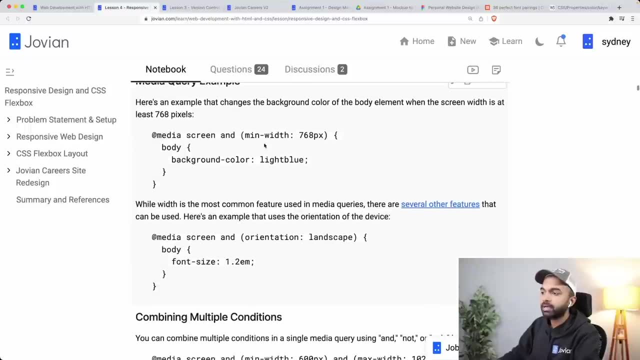 So if the condition min width of seven, 68 is met, So when the condition holds true, Then these CSS rules apply. Otherwise these CSS rules don't apply. All right. So here are some examples: min width, and you can also do it on orientation. 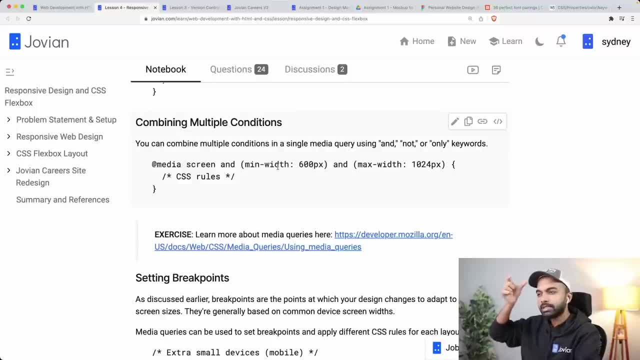 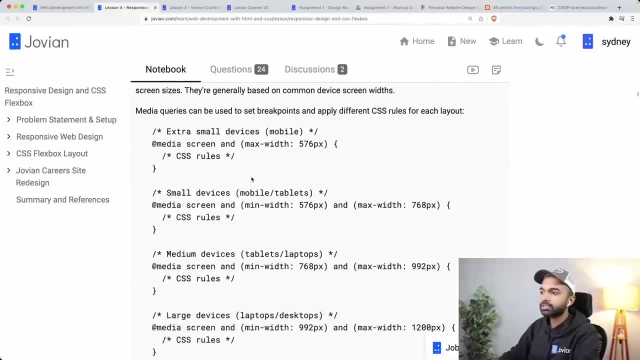 You can also combine min width and max width like that, So that way you can define specific rules for different windows of width. However, the better way to do it- So that's how you said, you can set break points, but the better way to do it is you use a mobile first approach, which is first right. 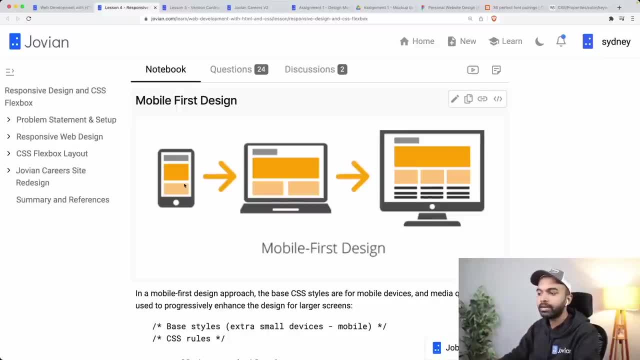 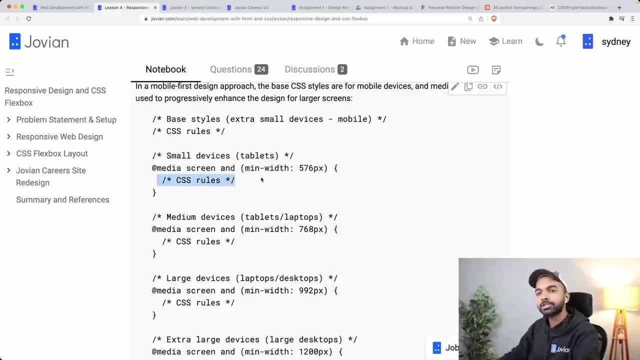 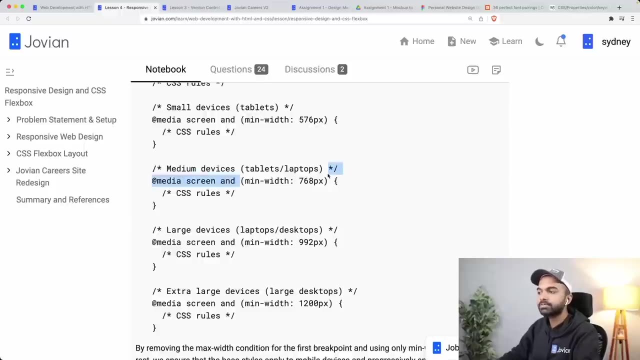 All your CSS queries or your create your design for mobile And then add, maybe for small or for tablets, add a min width break point and add some additional CSS rules that can go on top of that, And then, for your tablets and laptops, add some more rules by setting min width seven, 68 and so on. 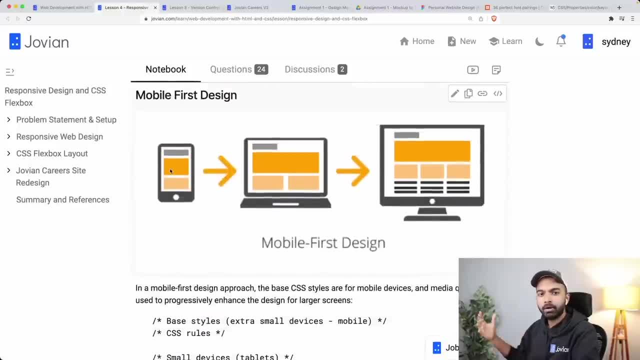 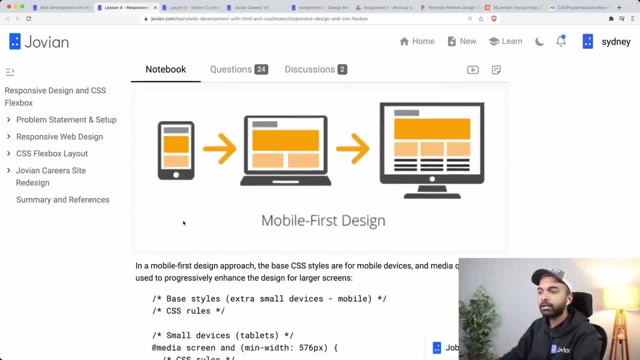 Right. So you want to ensure that you don't have to repeat a lot of the layout, uh, design, uh. and you want to start building from mobile first. So use this for your personal website as well. Uh, use a mobile first approach to start with the mobile design and then add. 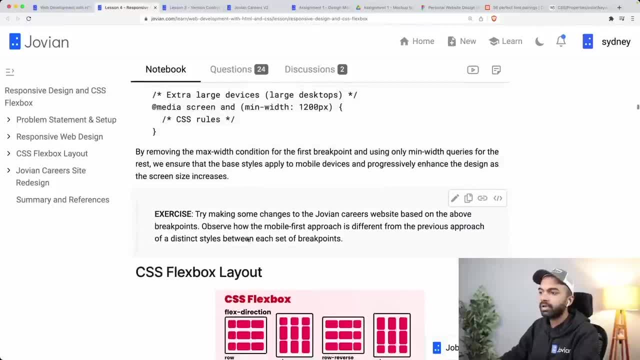 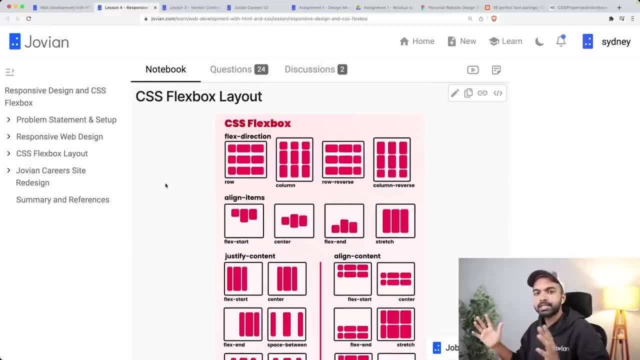 These break points, or you can use bootstrap to do it, Uh, but whichever way you choose to do it, this is um how you should achieve it. And we also talked about a flex box, because as browsers resize, you cannot exactly know what size you should build for. 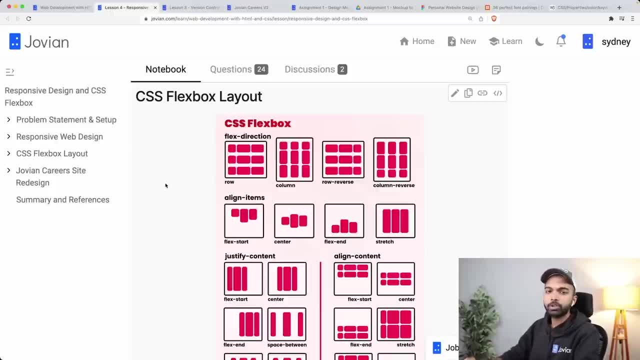 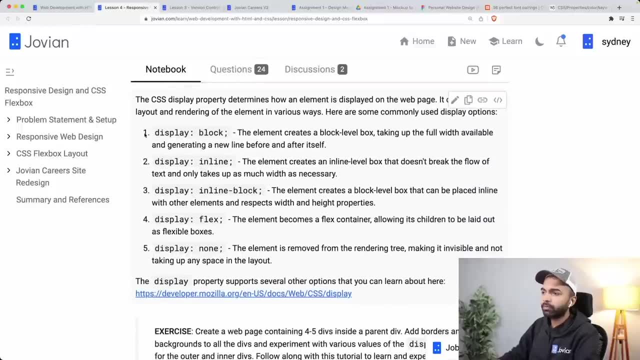 So you should- not, you should never- hard code your weights. but to keep your proportions constant you can use CSS flex box, And again, there's a bunch of things in CSS flex box. So the first thing is you have to set the display property. 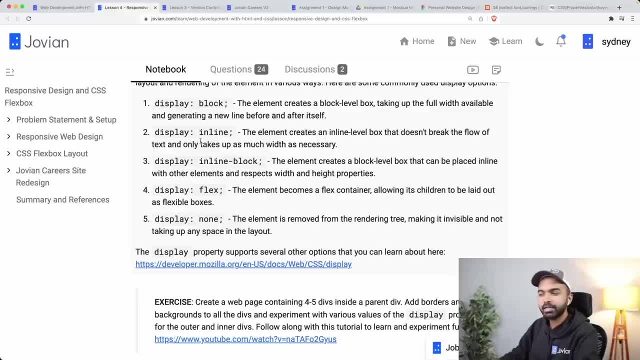 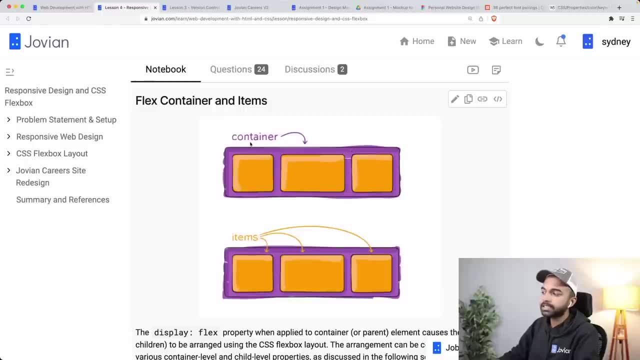 Now, of course, the block inline and nine blocker. Some of them, Yeah Yeah, They display properties, but display flex enables flex box and display none, uh, hides the element altogether. So flex box has this concept of containers and items. 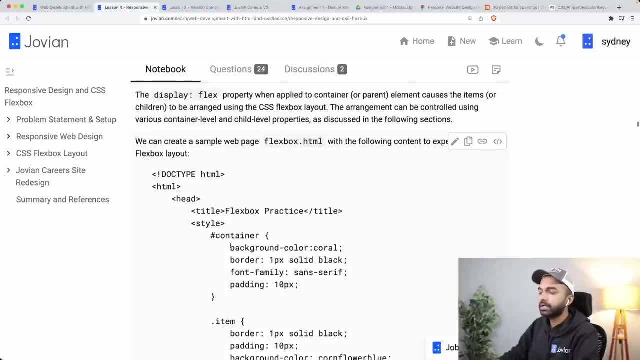 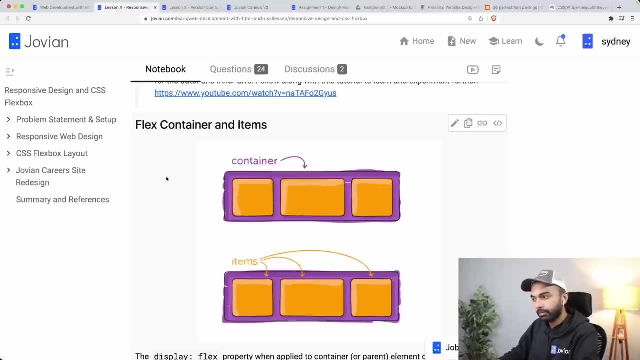 So there's a flex container and then there are a bunch of flex items. Now, uh, as soon as you said display flex, then the container, um, or the items, are laid out along. uh, according to the rules of CSS, flex box. 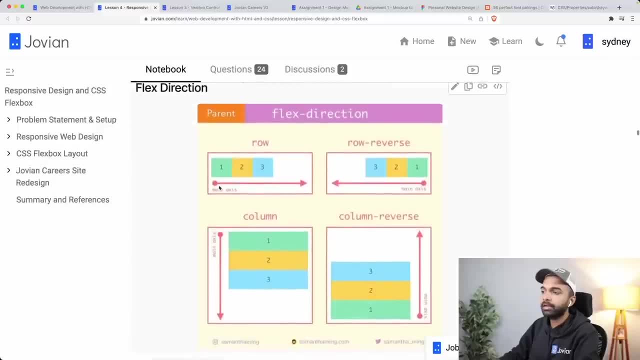 And then you can give a bunch of properties to items as well. So some are container level properties, Some are item level properties. One is the flex direction, Which is where things flow from left to right or right to left or top to bottom or bottom to top. 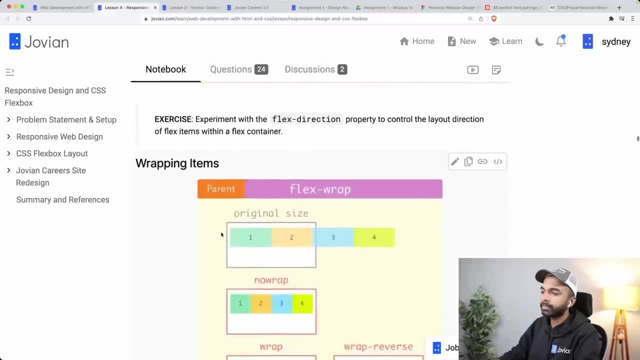 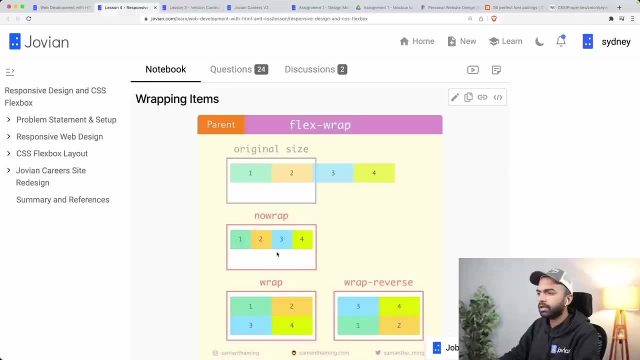 So this is done using row, row reverse, column, column reverse. then you have wrapping. So again, uh, things will by default just go out, But if you say no wrap, then they're going to try and fit or compress. um, you can say: wrap down, so they can wrap downwards. 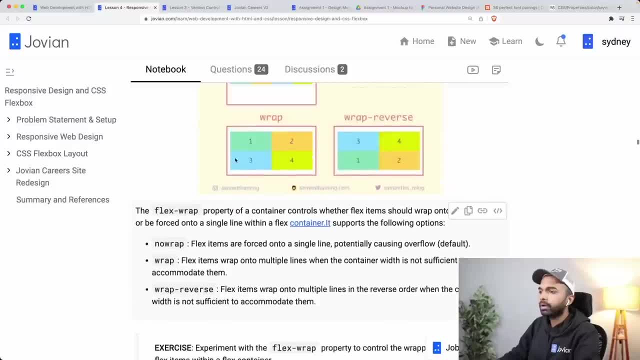 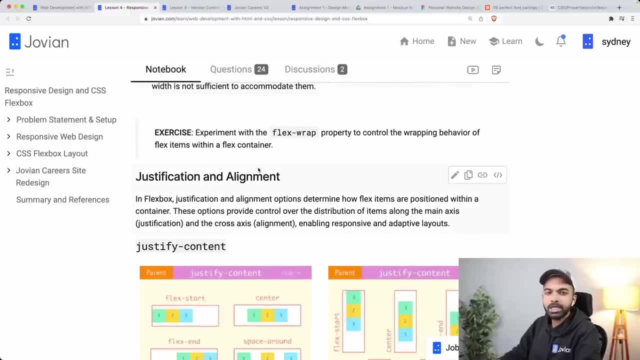 And you can say wrap reverse, and they can wrap upwards like that: Okay, Um, again, these change based on the flex direction, So you might have to just also, Uh, play around with it, but in most cases you just want to do the simplest thing. 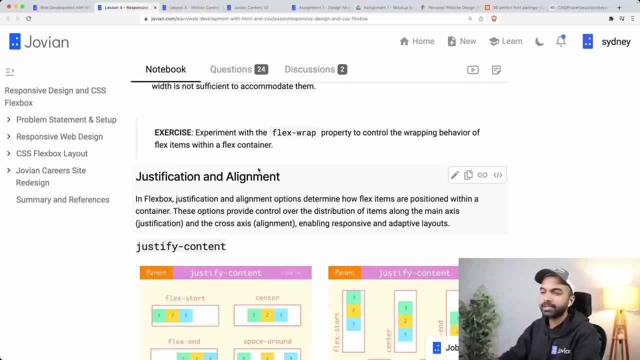 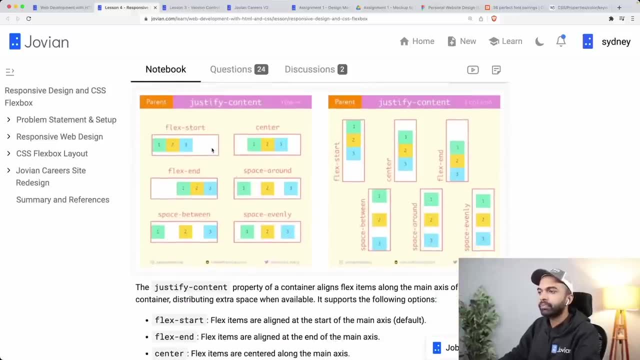 Some of these more advanced uh options never actually get used, or they get used simply when you're trying to achieve a fairly advanced layout, which doesn't really come up very often. So then you have justify content. So, along the main axis, do you want things to be at the start, at the center or at the end, or maybe you want to be spaced? 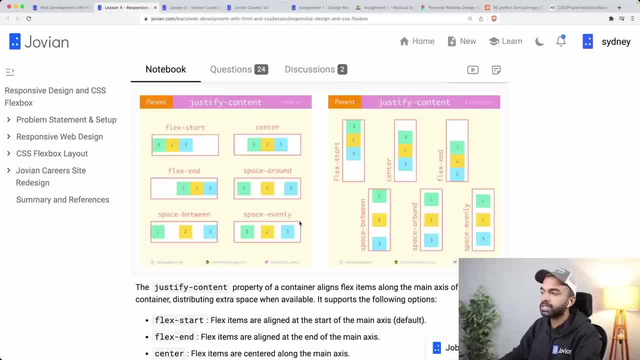 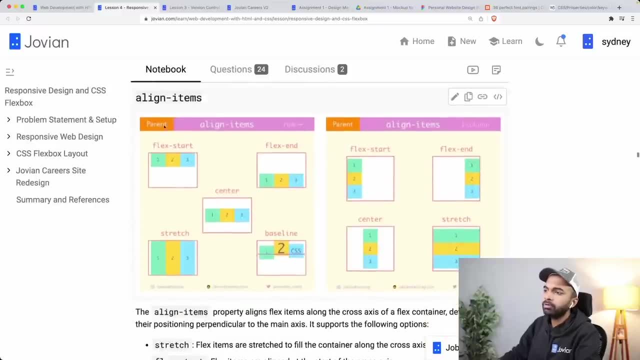 Um, you want space around them, You want space between them, or you want even spacing, or uh, and of course for uh, flex direction column, It's going to be different. Then you have align items, and that applies along the cross axis. 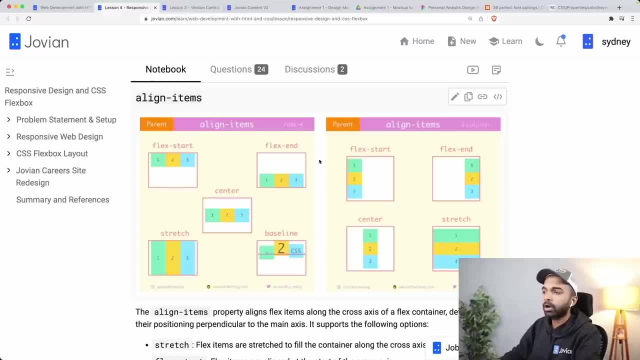 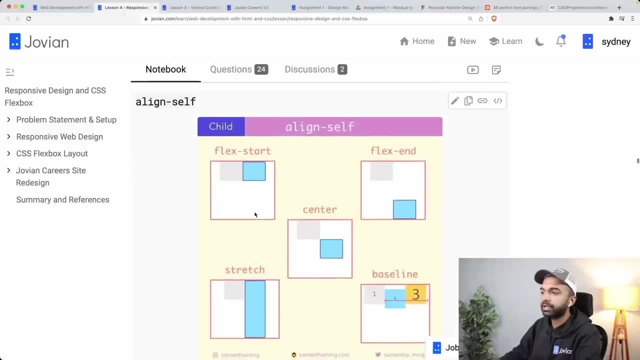 So again, if the flex direction is row, do you want things to be sticking to the top, sticking to the bottoms? uh, be at the center, or stretch to take up the entire space, or maybe align according to the baseline. So that is something that you can look at as well. 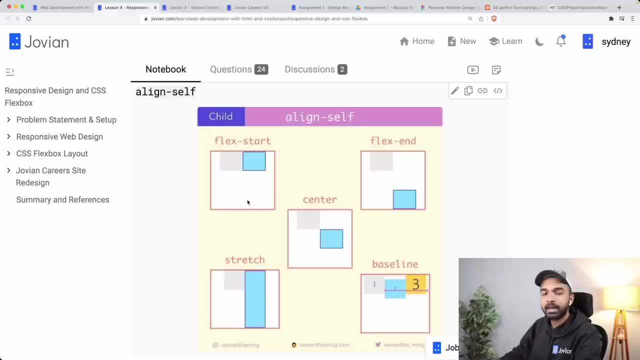 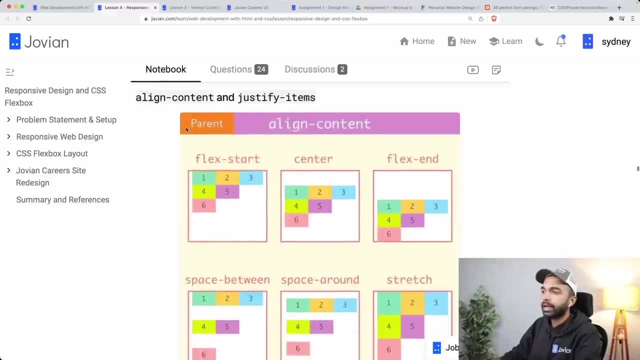 Then you can change the alignment at a child level as well. So let's say you have an alignment setting at the parent level, You can actually modify that setting for a particular child using the align self property And you also have something called align. 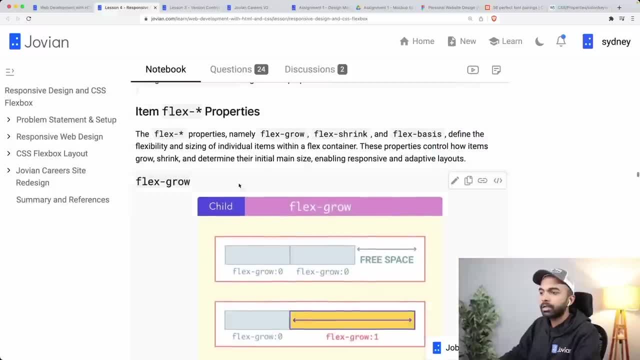 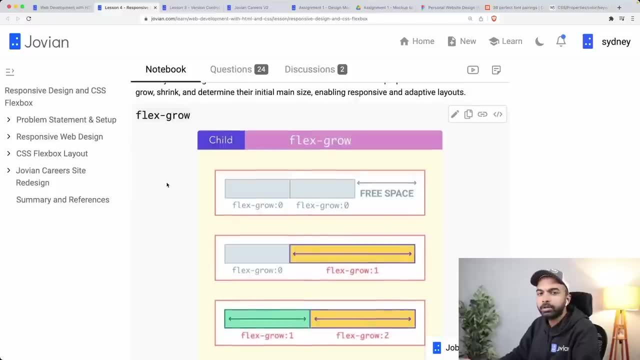 Content just by items. I've almost never used them, So I wouldn't worry about it. You also have these properties: flex, grow, flex, shrink, flex basis. They have a certain meaning. I would really not bother about these too much. 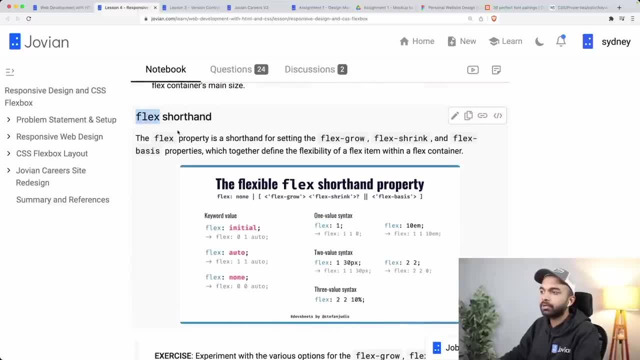 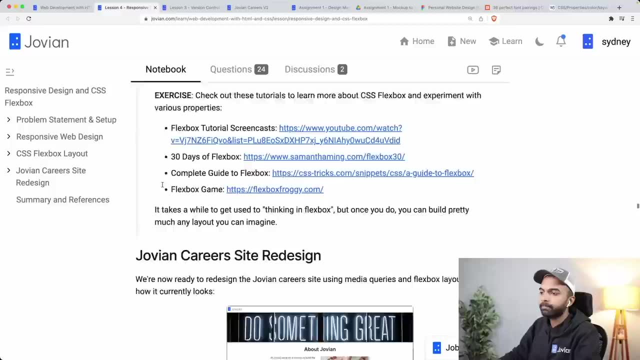 Really, The only property that I often just use is the flex property, where I would just simply put flex one to make something. uh, take up a bunch of space, uh, all the available space, Okay, So that is that, and using that, we then decide that we want to redesign it using a flex box. 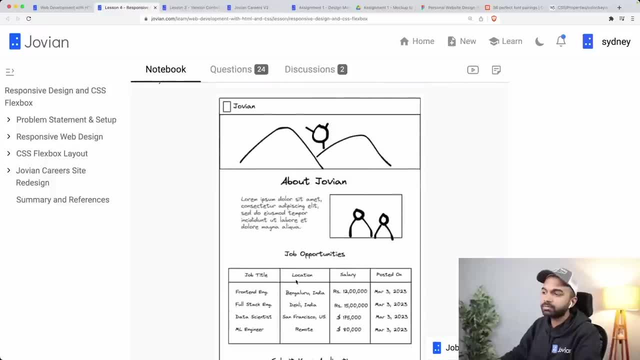 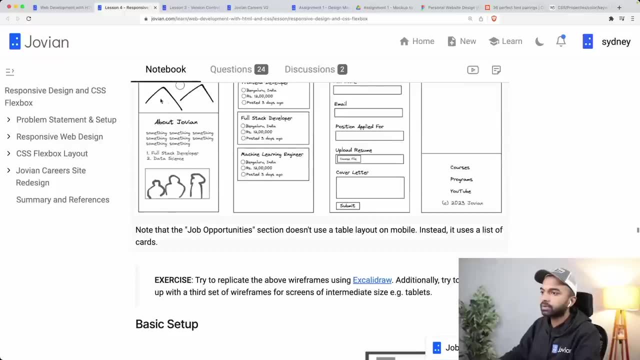 So we, the first thing we do is we create a couple of wireframes. We create one wireframe for desktop and we create one wireframe from mobile. So this is what we want it to look like on desktop And this is what we want it to look like on mobile. 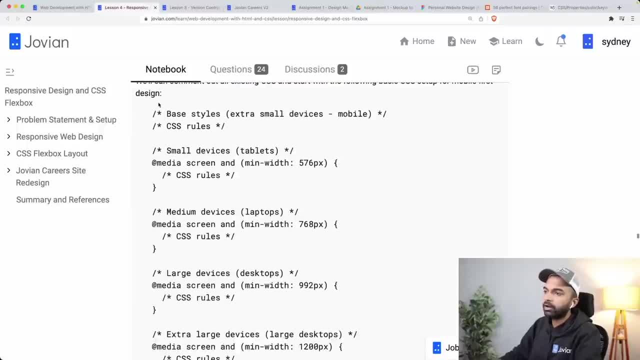 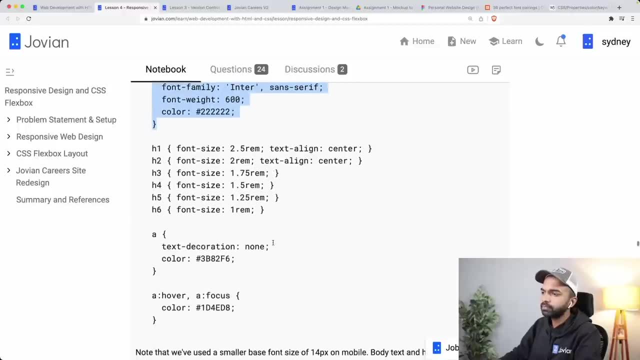 And we start with a mobile first layout. So we lay out a bunch of base styles and we- we have a base font size, We have a base body size, We have a base um uh, we have a base size. We have a base heading sizes. 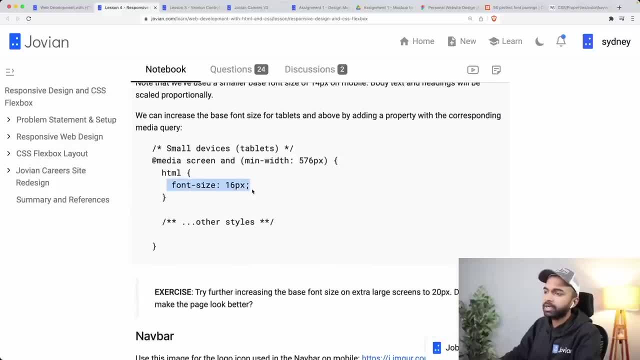 We have, uh, we have, a bunch of base styles and then, Uh, for tablets, we want to slightly increase the body font size and so on, Right, So, yeah, so we, then we create that nav bar, uh, like this: 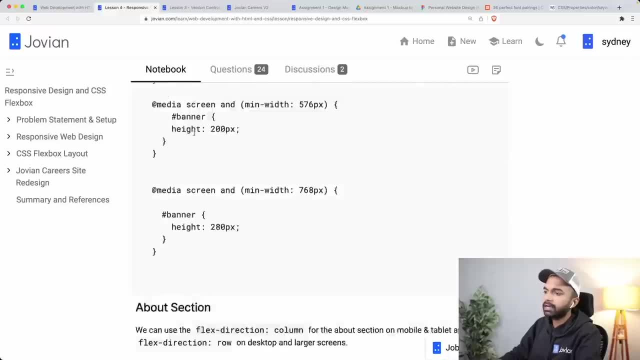 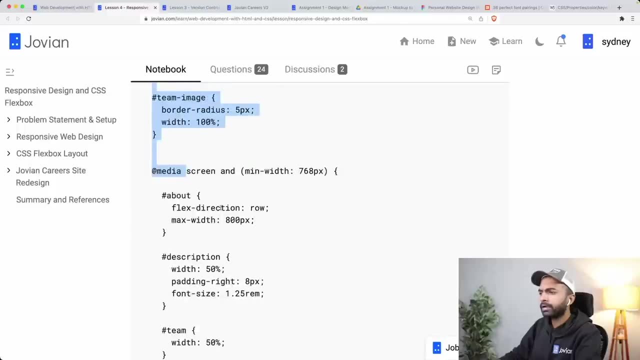 So for the nav bar we use a slightly different logo. Then we created the banner image, We created the about section and then we added: we started with a mobile first layout And then we added a bunch of things here to change the layout slightly on mob, on tablet and on desktop. 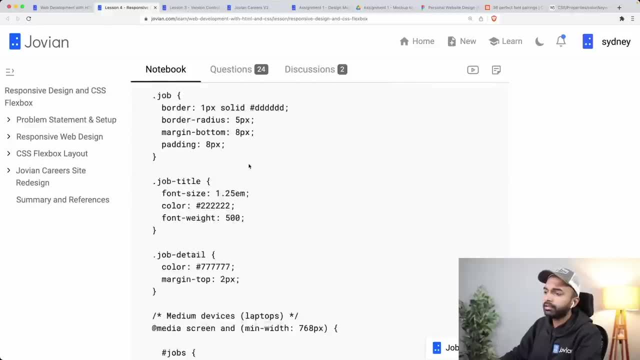 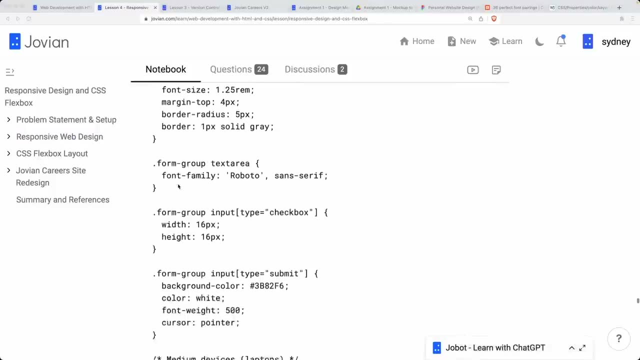 Then we have a jobs list that was shown on mobile and tablet, and then we have a jobs table that is shown on desktop- So Yeah, a jobs table that is shown on desktop- And then we have this application form. We made some changes here, but ultimately this is what it looked like on mobile. about 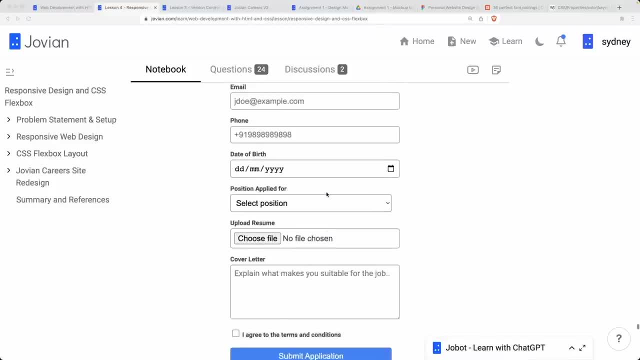 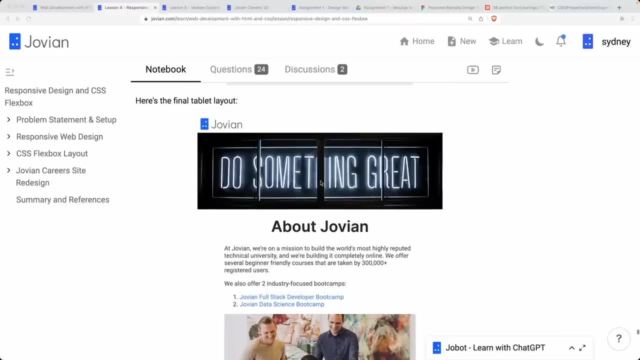 Jovian employment opportunities, submit your application, et cetera, et cetera. Uh, it looks good, It looks readable. uh, could be better, but it looks readable. And even these are stacked vertically, and this is what it looks like on tablet, slightly different. 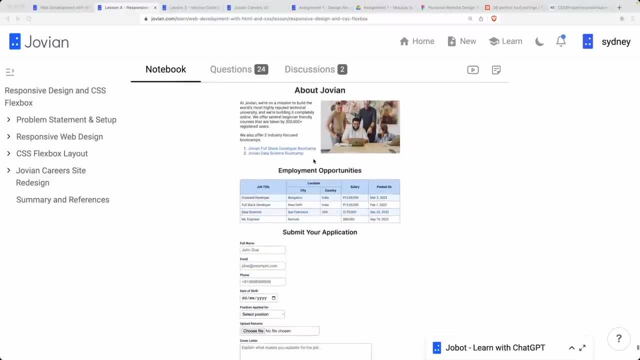 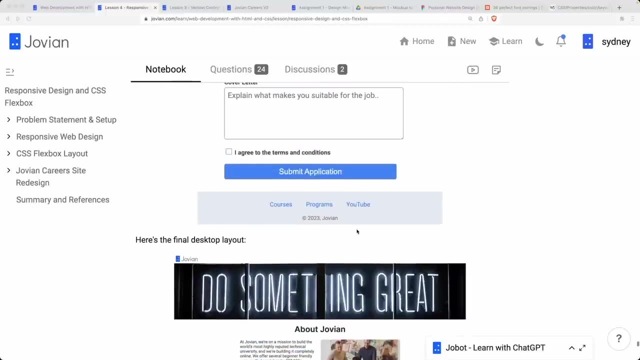 Okay, Slightly more spaced out, but still using the list. And then this is what it looks like on desktop. here It's using a table And here the three footer items are shown vertically, are shown horizontally like they are on tablet. 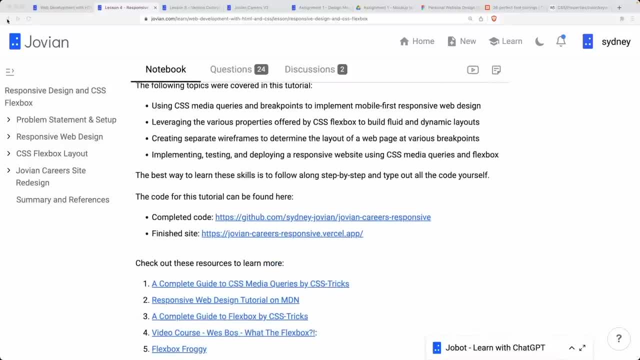 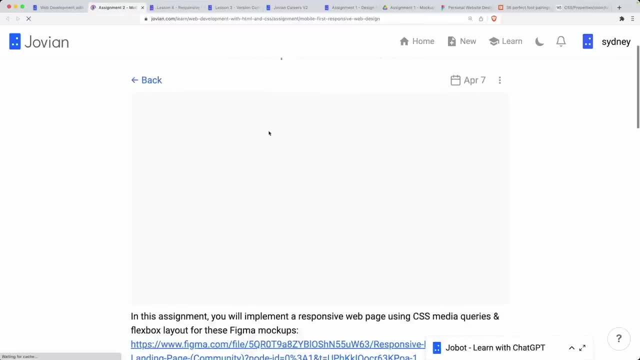 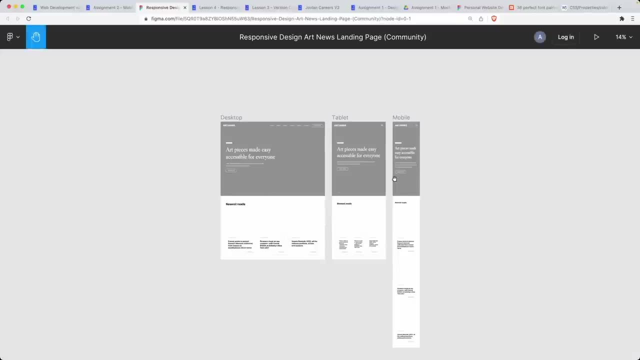 Okay, So that's our- uh, that was a lesson on responsive design and CSS flex box. Then we hired an assignment on mobile first responsive design where you had this layout that you had to implement. So this was the layout where you had a mobile tablet and desktop layer and you had to implement each one of these like that. 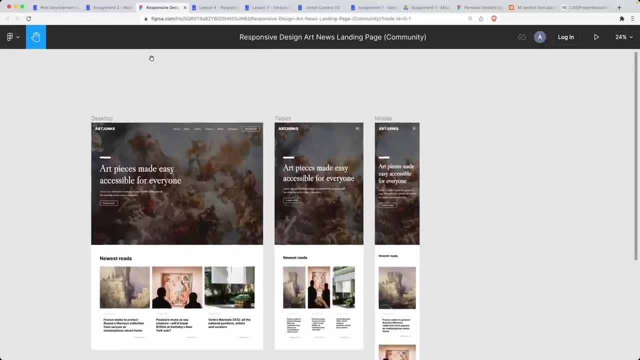 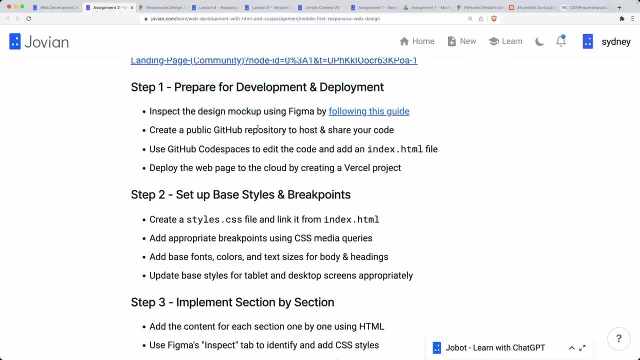 And Yeah, I think there's not much to be said here except that you could use flex box to do this, And you also learn about the CSS Calc property. And these are the the process you first set up: prepare for development and employment. 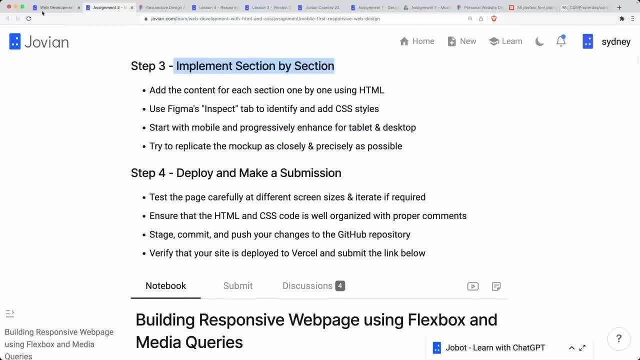 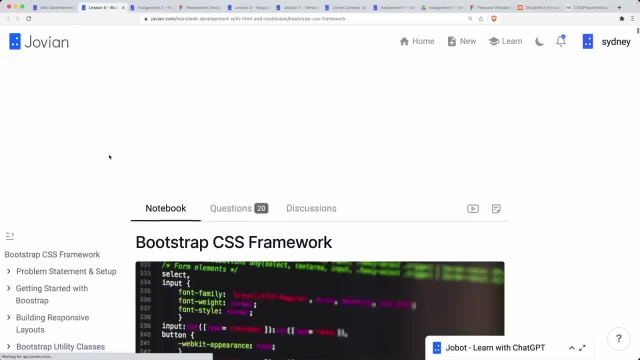 You set up base styles and Blake points, implemented section by section, and then you deploy and make a submission. Okay, Then we learned about the bootstrap CSS framework, which is, uh, which makes life really easy when you're working with, uh, when you're working on a complex project. 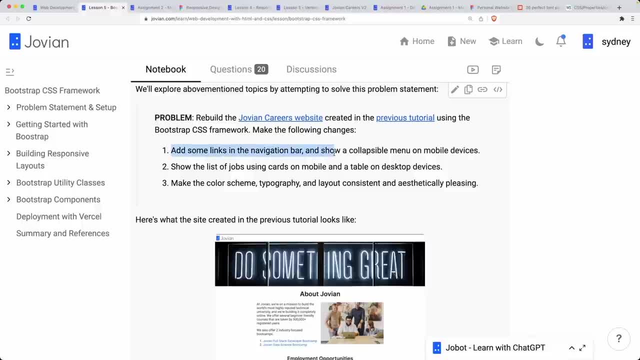 So again, we wanted to rebuild the Jovian careers website. Add some links in the navigation bar, show a collapsible menu on mobile devices, show a list of jobs using cards on mobile and table on desktop, and make the color scheme, typography and layout consistent and aesthetically pleasing. 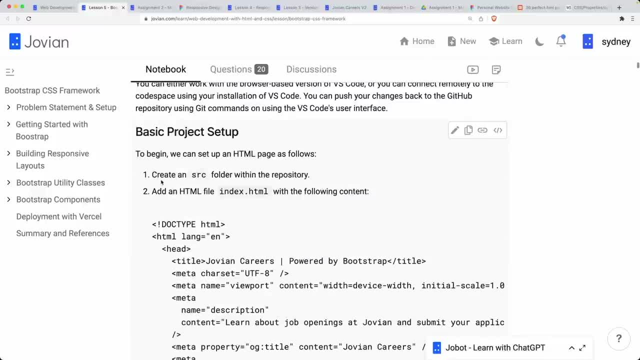 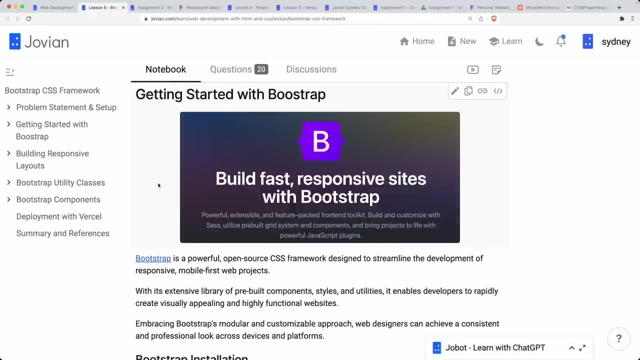 And for that we wanted to use the bootstrap. So there's a basic project set up, of course, but we wanted to rebuild the project using bootstrap. A bootstrap is a powerful open source CSS framework that is used to design a streamline the development workflow, especially for mobile first designs. 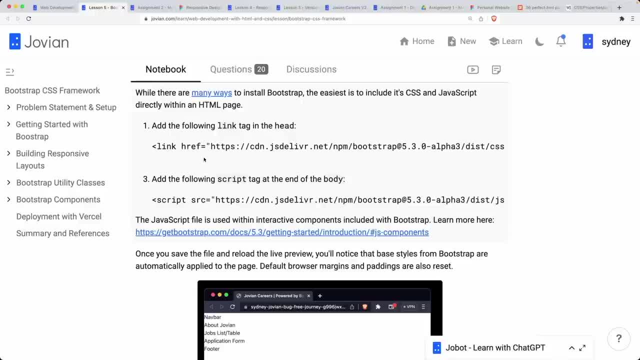 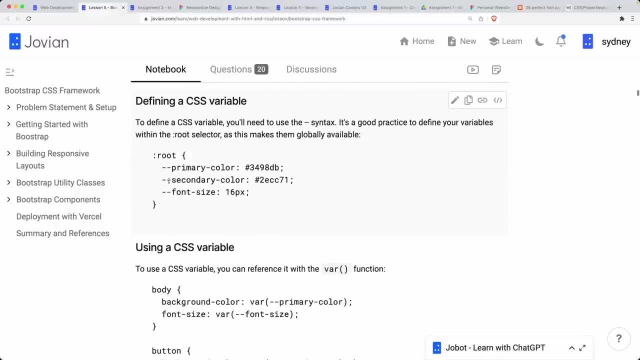 So we installed bootstrap, and we installed simply by including a couple of links within our page and right right away, changed a few styles. Then we customized it using CSS variables. So we changed the primary color, We changed the- uh, let's see. 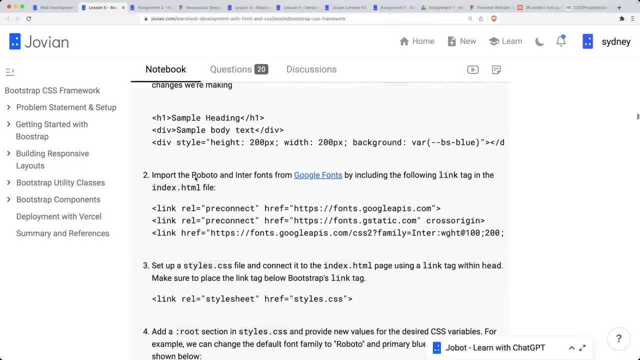 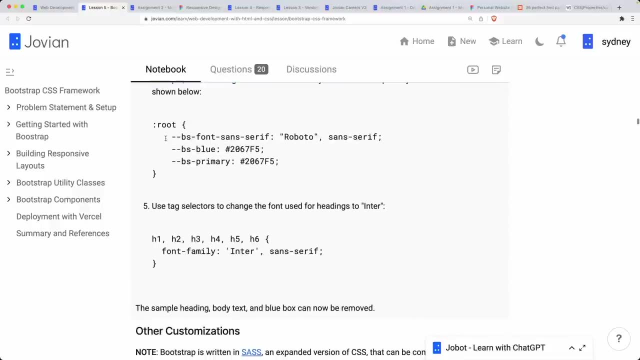 Yeah, So we changed customized bootstraps, typography, We customized- uh, we customized the fonts, So we used a couple of outer fonts. Then we created a status or CSS file. We said the fonts, we said the primary color and we said maybe the heading. 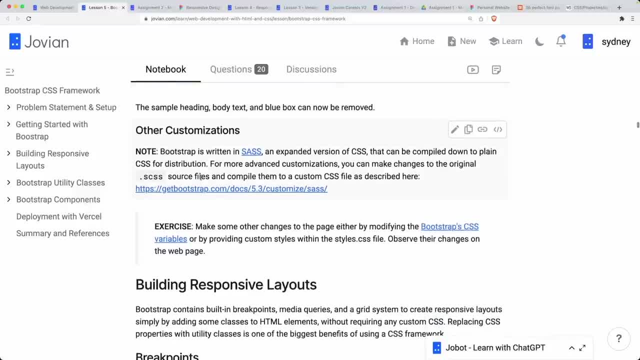 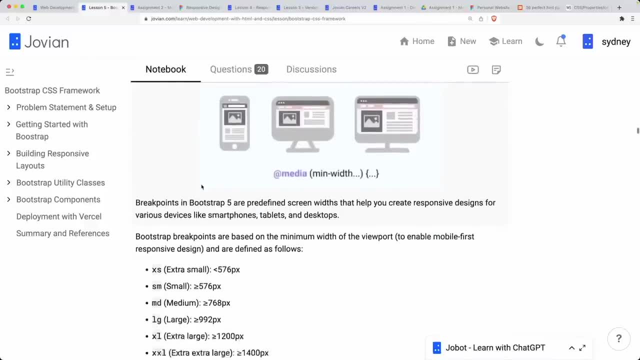 Okay, We want to be entered, and there are other customizations that can be done, but these basic customizations should do the job, even for your own personal website. Then we decided that, okay, we're going to start out. So bootstrap has a bunch of pre-configured breakpoints. 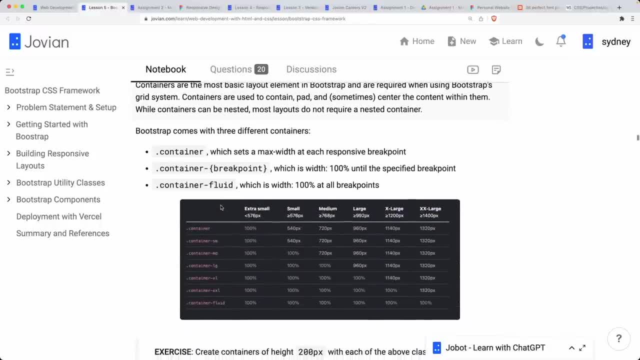 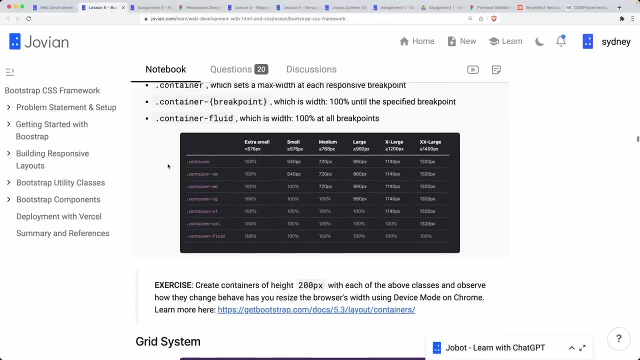 So we're going to start out with, uh, just building out a basic container and building out a layout and then making it responsive by adding more utility classes. So in bootstrap you're typically started with a container that centers your content on the page horizontally. 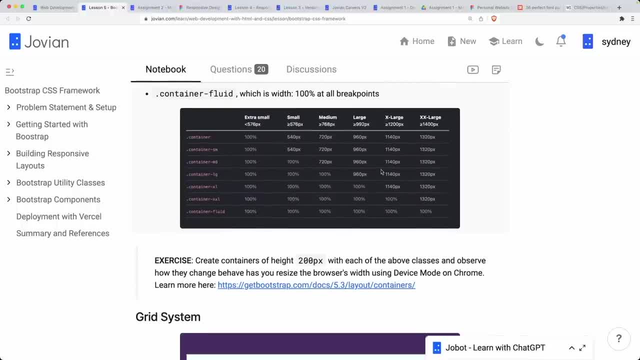 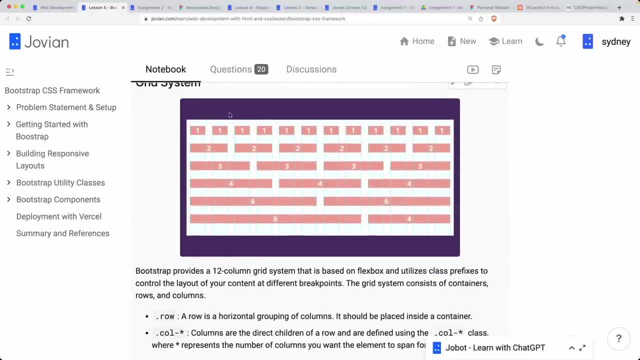 And it takes up full width until whatever size you want, And after that it's a stays in the center and bootstrap has a grid system, a 12 column grid system, And what you can do is you can uh set up a row and inside that row you can have a bunch of columns and you can set weights for those columns on how many of these uh grid elements you wanted to span. 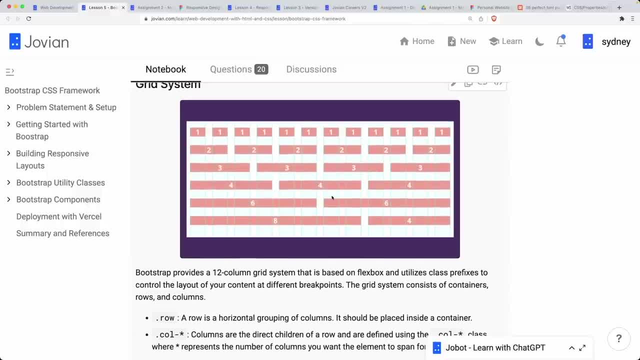 So you can mix and match. You can have three, three, three, three, or you're going to have three, four and four, or you can have maybe three, three and six- You're going to have three to do things like that. 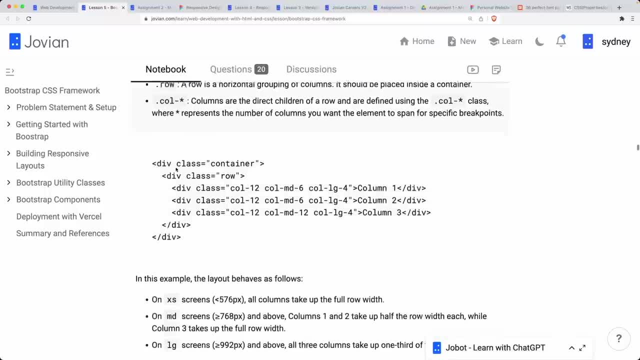 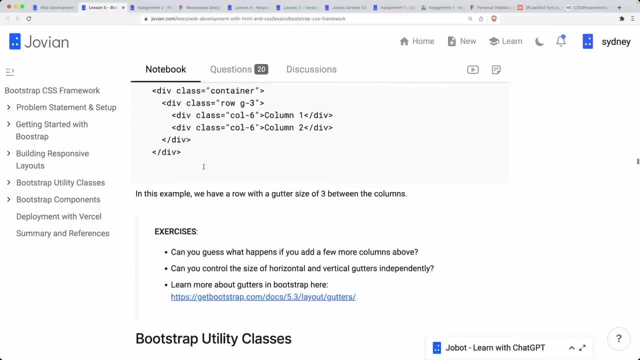 As soon as it crosses 12, it goes onto the next row. Okay, So you create a row and inside the row you create a column, and that's what it does, And then we talk. we looked at offsets, We looked at gutters. 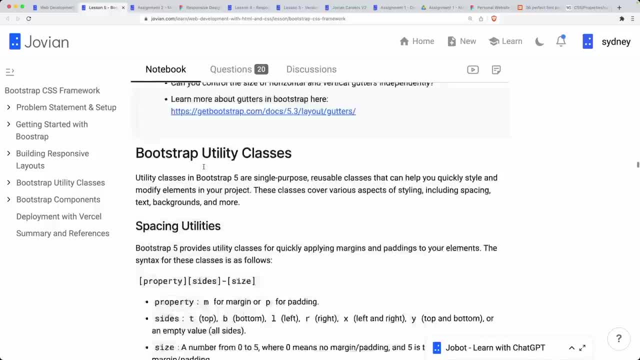 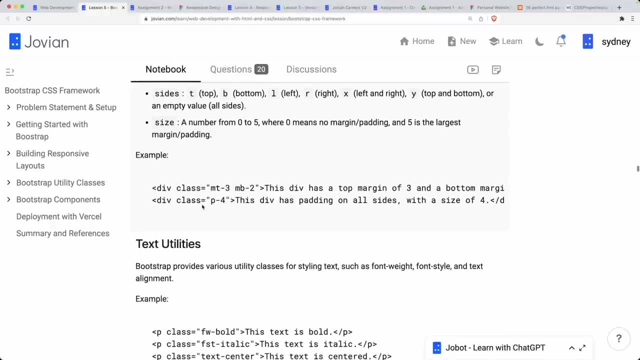 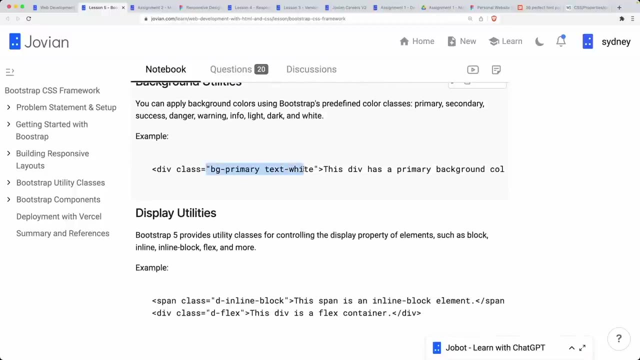 Those are just ways to shift things around here and there. And then we talked about utility classes. So bootstrap has a bunch of utility classes to set margins, set paddings, um, to set sizes, a bunch of utility classes to make things bold, italic, to center text, a bunch of utility classes to set background colors, a bunch of utility classes for borders, for display, for 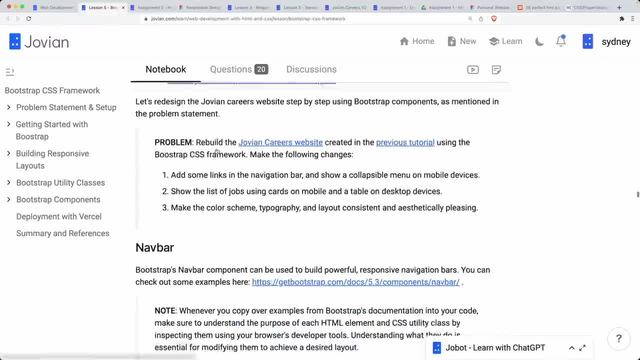 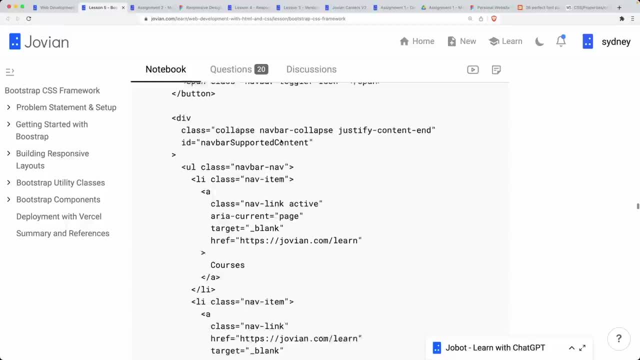 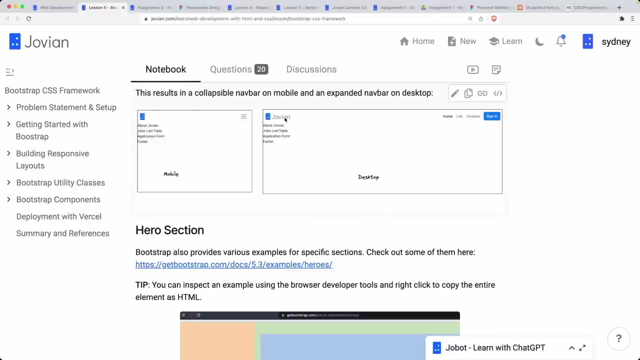 flex, et cetera. Okay, And it also offers a bunch of components. So it offers a navbar component so you can use something like this. Um, so this is a navbar component for our site And this produces a navbar like this, which on mobile, created a collapsible menu, but on desktop creates this nice three links with a sign in button. 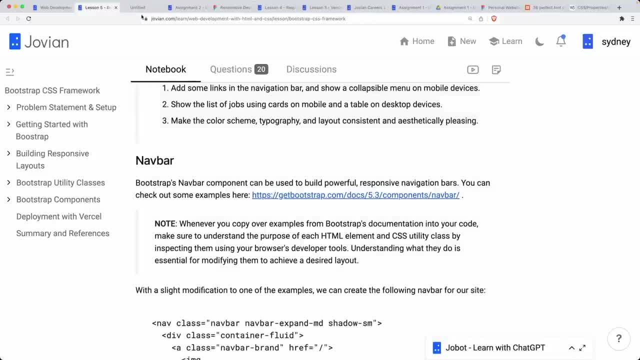 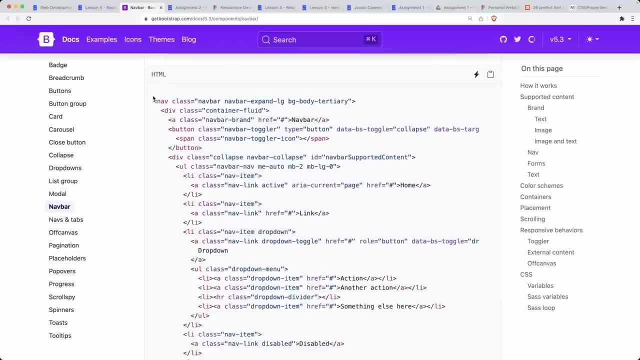 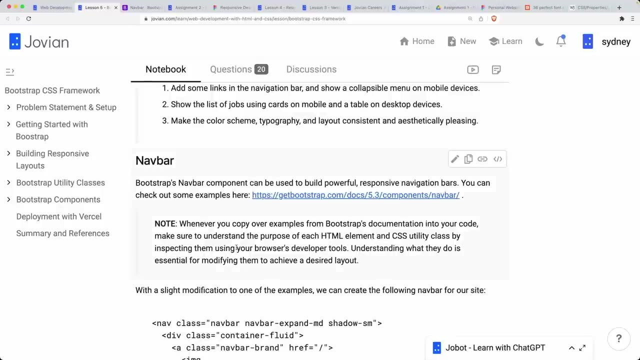 So what you do typically with components is you check out the example code and you simply copy paste and drop it into your um. not copy Paste exactly, But yeah, take a close look at it and either just drop it line by line or write it, or maybe in some cases, when it's exactly what you need, just copy pasted and it's fine. 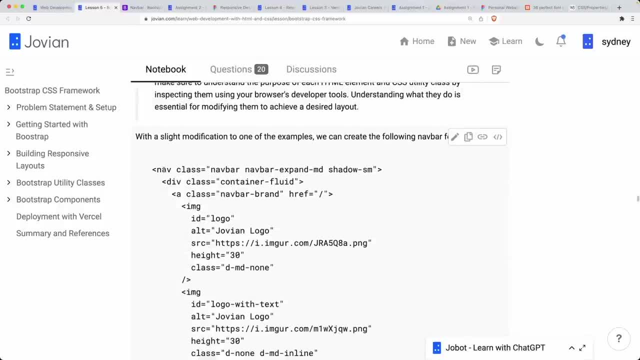 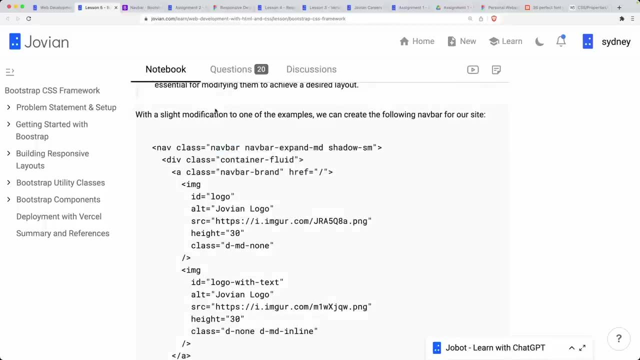 But make sure you understand every line of code that you're copy pasting. Don't have anything that doesn't actually make sense. You can always inspect something. You can right-click inspect on the page itself and see what exactly a piece of code does. 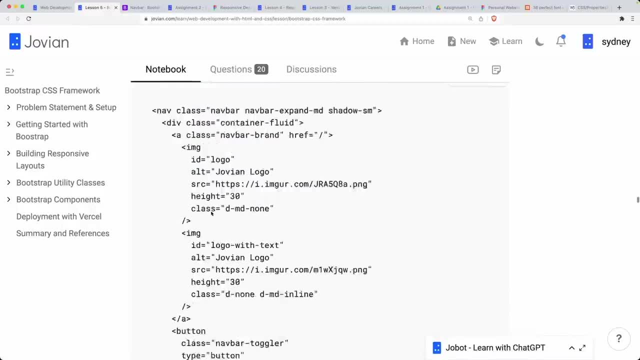 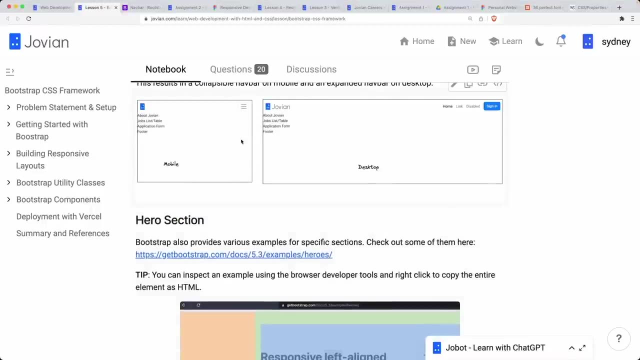 Okay, So that's the navbar over here. It had a couple of images, So we were using a different logo on mobile. Okay Okay, Different logo on desktop. like that You can do all those using some utility classes. Then we created a utility hero section. 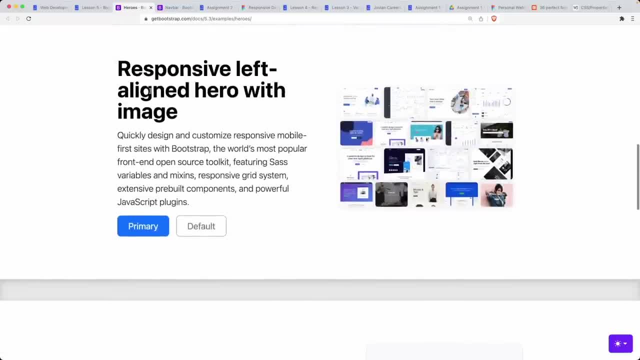 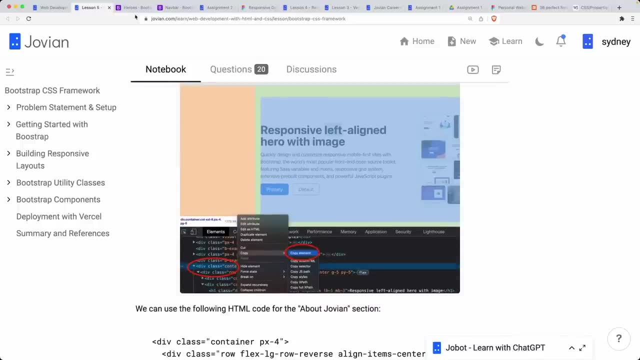 Again, there are a bunch of examples here for the hero section, and we found this one interesting, So we went ahead and simply copied it from the browser itself, So you can just open up these tools. So, again, feel free to use some of these examples. 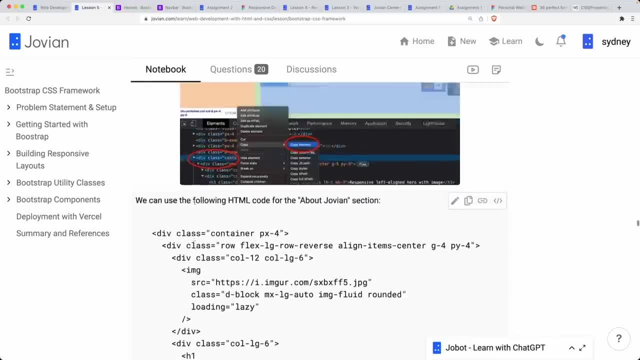 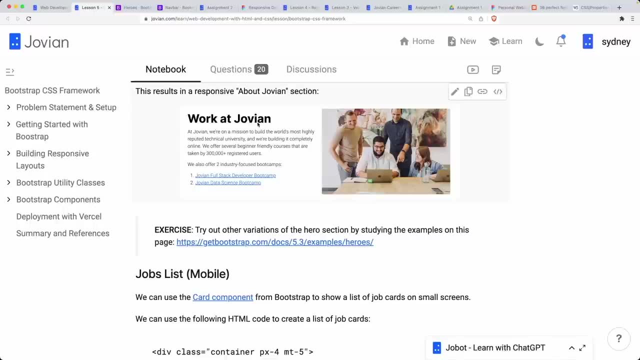 If you think that is going to be useful for your website, your personal website. and then we pasted it in here and made some changes And we got this nice hero section which looks pretty good, Pretty Well designed, And yeah, that's with that. 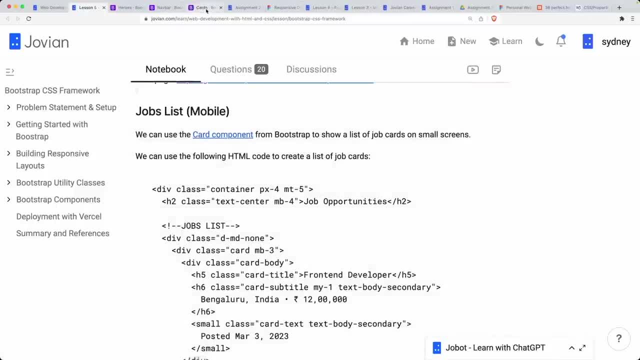 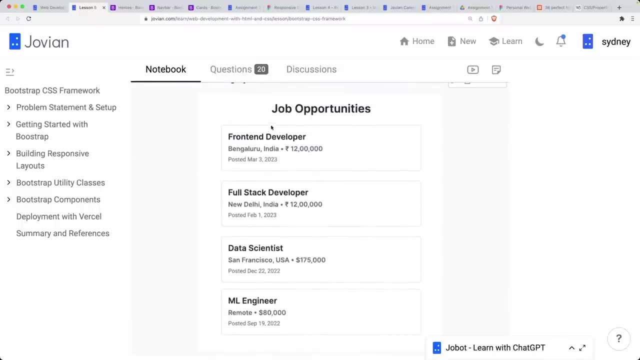 We had the hero. Then we created a jobs list. This is where we used a card component. So bootstrap has this card component that we could use. So we added a bunch of cards and you can see here that we created this nice job opportunities and it has this nice visual hierarchy: big text, bold font, dark color, smaller text, then even smaller text, lighter font, even smaller text, even lighter font. 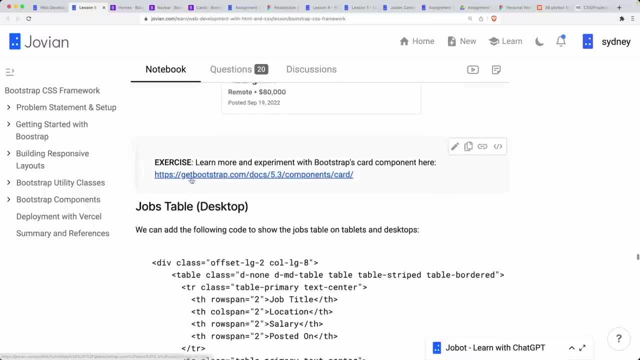 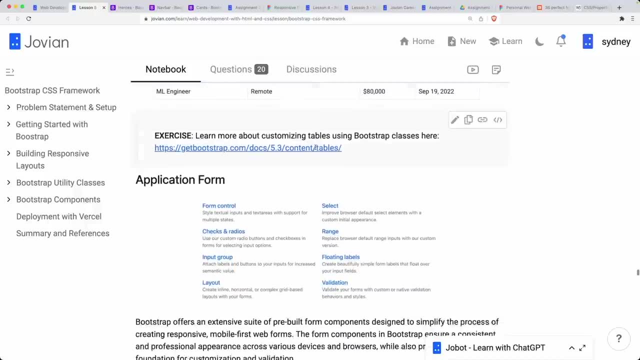 Right, So use all of these things to give your content some hierarchy. Then we created a jobs table for desktop- Again, bootstrap has some examples of creating tables, and this is the table that we ended up creating. Then we wanted to create a form. 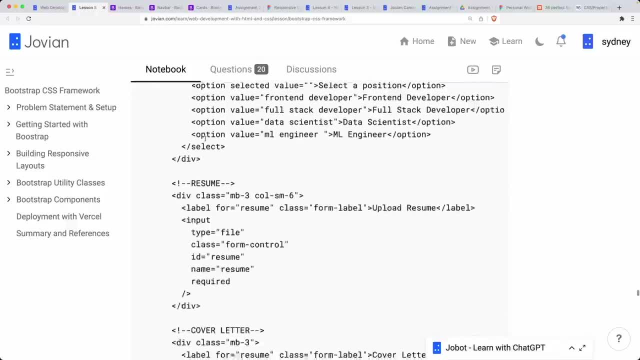 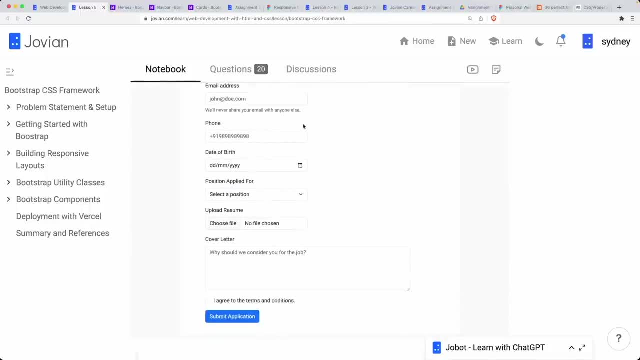 And again, bootstrap has a bunch of great utilities for building forms. So we just dropped in a bunch of examples and then modified it And that gave us this nice little form with everything looking very consistent, very clean and also a nice submit application button. 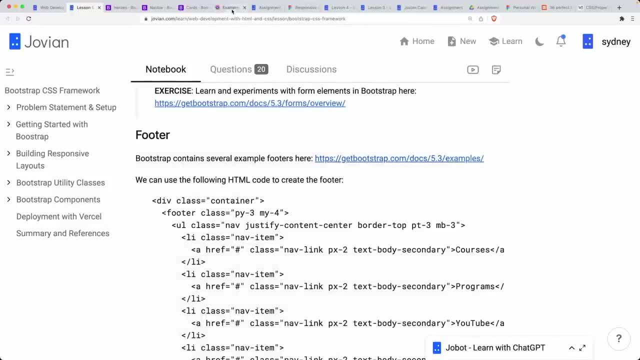 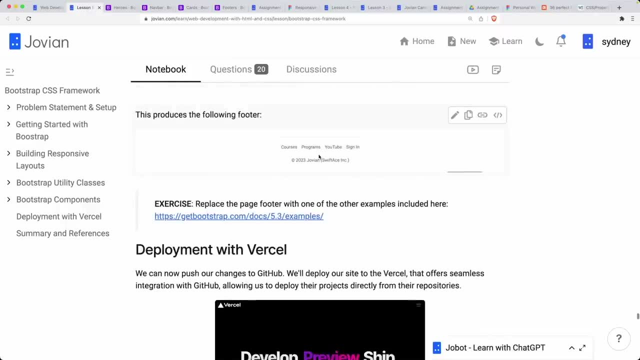 And finally, bootstrap. we looked at some examples for footers over here, Like, for example, you have a bunch of Footer examples. So from this we picked out an example that worked for us and we added a footer as well, And, and. then we took the site and then we deployed it. 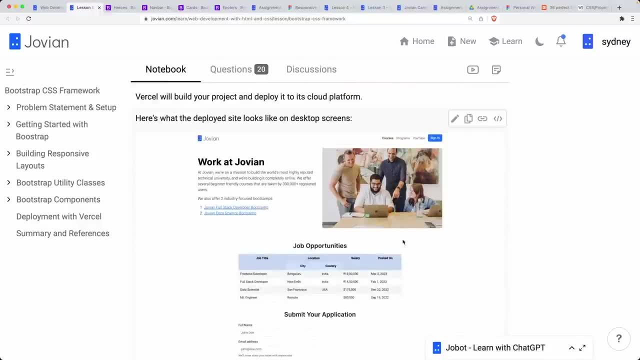 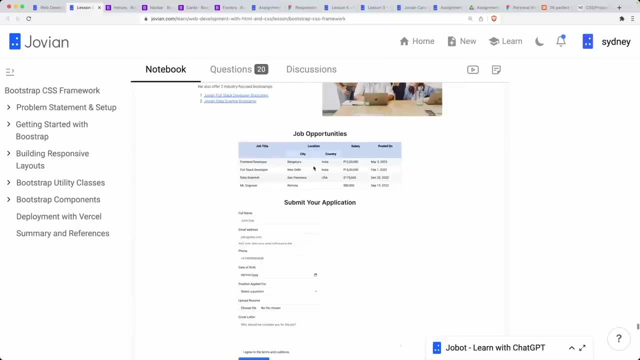 And this is what our site looked like, which is so much nicer. It looks so much cleaner And, if you want, you could just use a bunch of these bootstrap components and templates to build out your personal website and make it look just something as simple and clean as this. 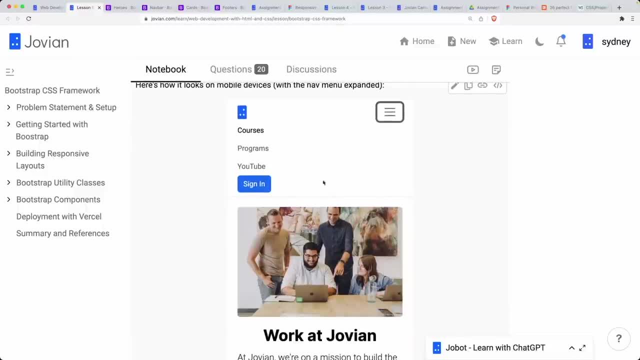 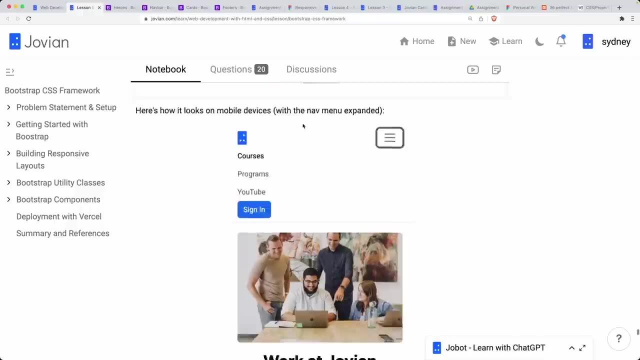 And that's perfectly fine. That's not a problem at all. And this is what it looks like on mobile: this expanded menu and then work at Jovian. Some of the content Is centered And, of course, things that were side-by-side have come one above the other. 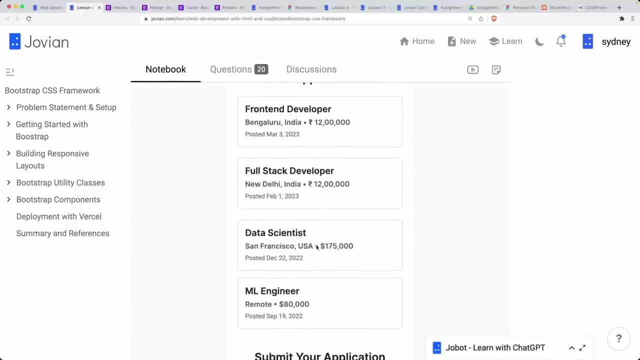 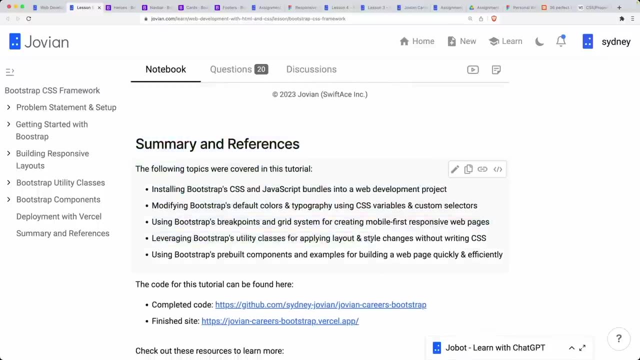 The table has shifted and now has gone away, And now we are showing a bunch of cards. Then we have the submit application section and that's it, And then we have summary and references about this and a bunch of tutorials on bootstrap that you can check out. 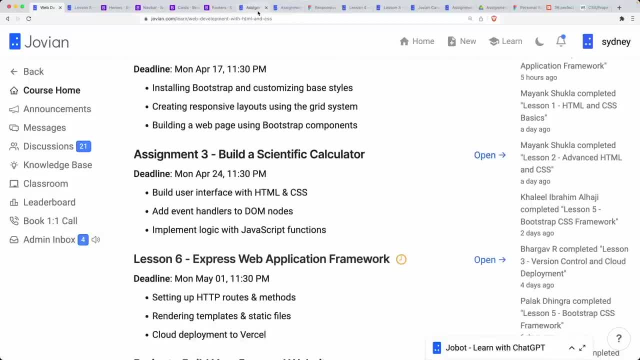 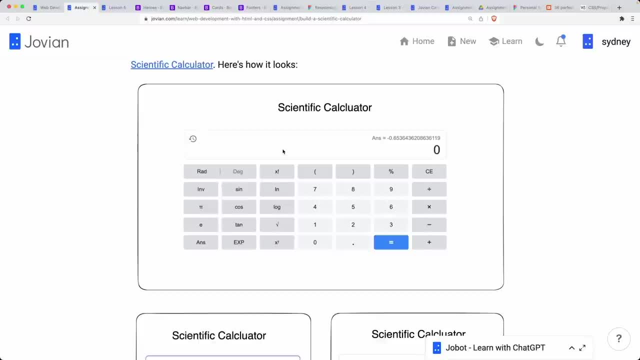 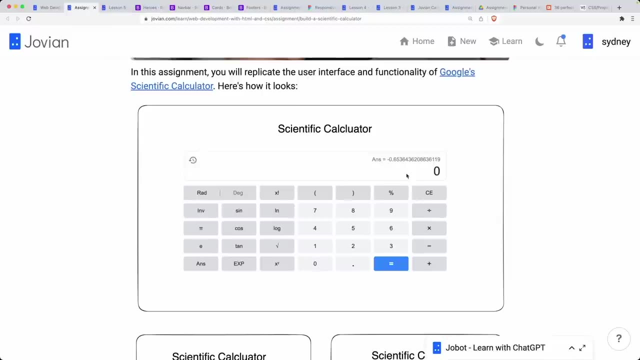 Okay, So that was a bootstrap CSS framework, And the next assignment was building a scientific calculator, And here your job was to use Not just HTML CSS but also some JavaScript to build out a scientific calculator that is as similar to Google scientific calculator as possible. 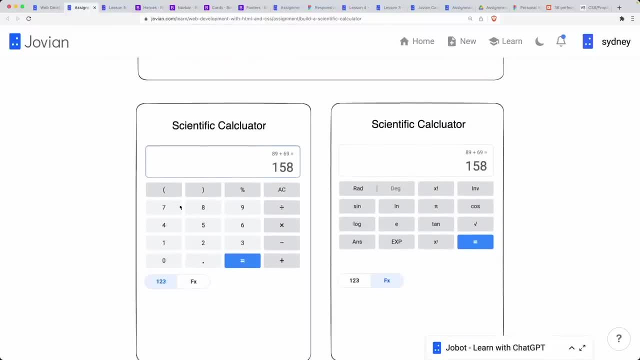 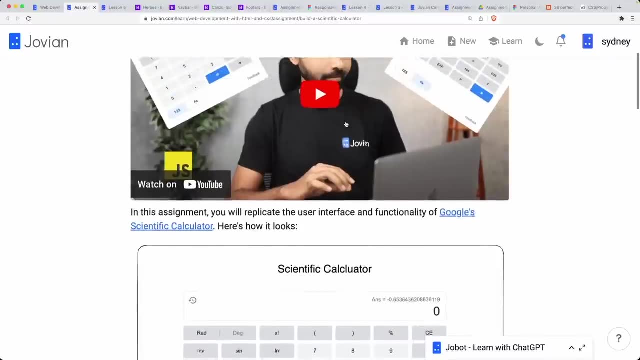 And many of you did a pretty good job at this, And you also wanted to make it responsive, so that it looks like this on mobile And it looks like this on desktop. And there's this tutorial here that goes into how exactly you add the JavaScript functionality. 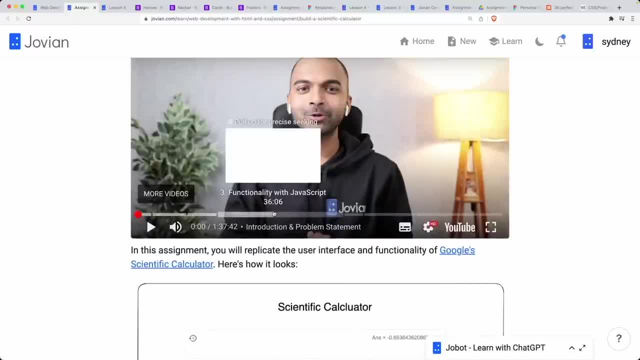 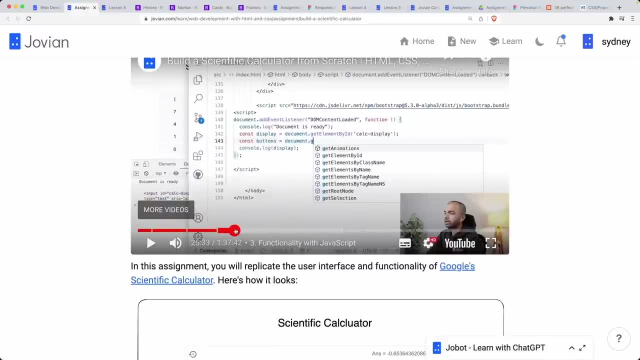 Yeah, basically, what you do is: let's see, you go in here, you add in a A bunch of event listeners for each of the buttons and for each of the buttons. you, yeah, you, you add event listeners and then you add the logic that you have. 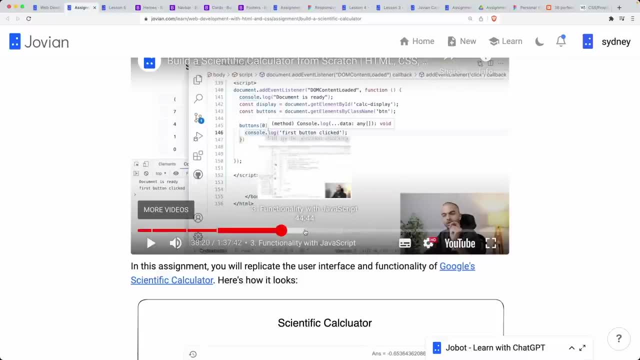 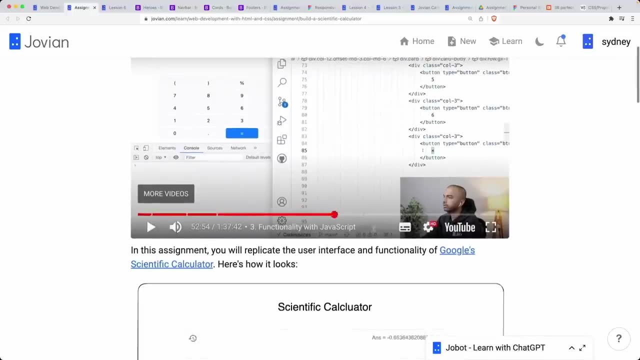 Maybe you take the expression and then you evaluate it or you add something to the expression. All of that is covered here. I think there's a great tutorial on how exactly to use JavaScript to add interactivity, And we are going to go much deeper into adding interactivity, but for now, I think this, this, does the job. 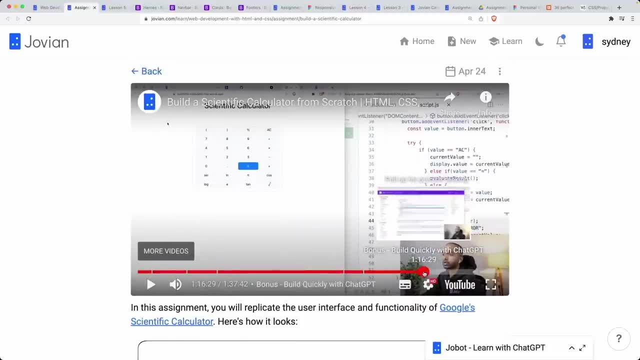 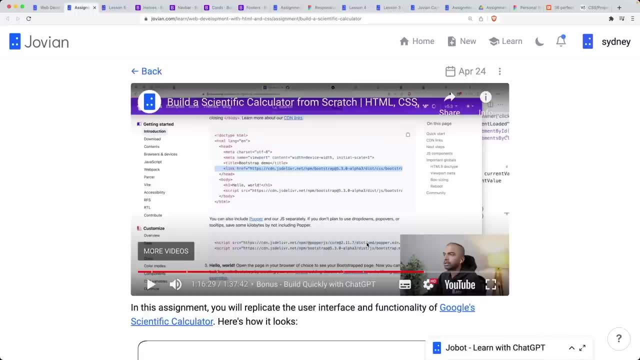 And the last thing I want to mention is you can build these things pretty Easily with chart GPT. Anytime you want some piece of functionality on your beach, you can always say: let's say, how do I animate some text to just shift up and down as um this user is scrolling. 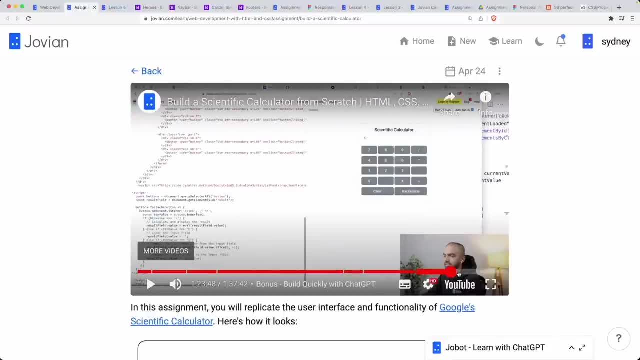 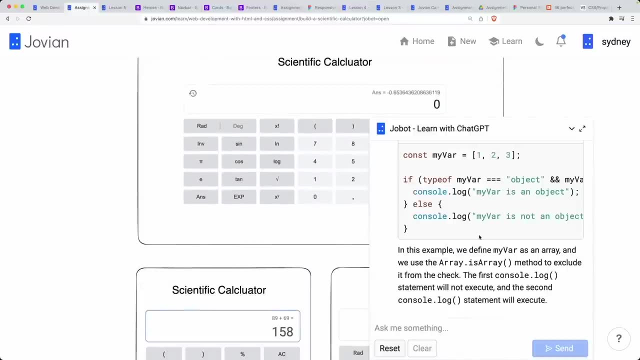 You can always just search on chart GPT and get some uh code from it, Right? So that's what uh? I just want to mention that as well. use chart GPT or use job bot right over here. Use your bot for help too. 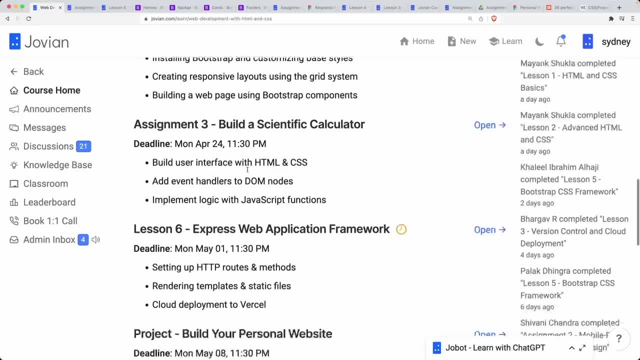 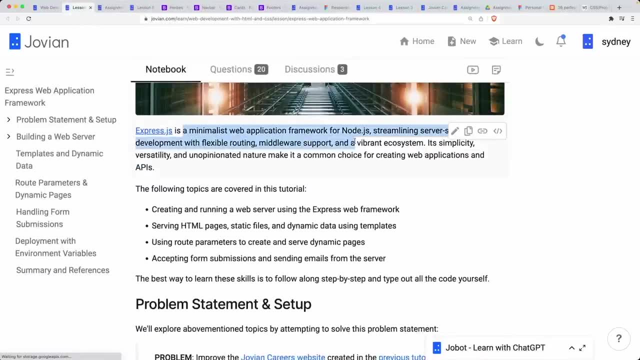 Okay, So that was the Um Assignment. Then we talked about the express web application framework. So the express web application framework is a minimalist framework for node JS for streamlining server side application development, with flexible routing and middleware support and a wide brand ecosystem. 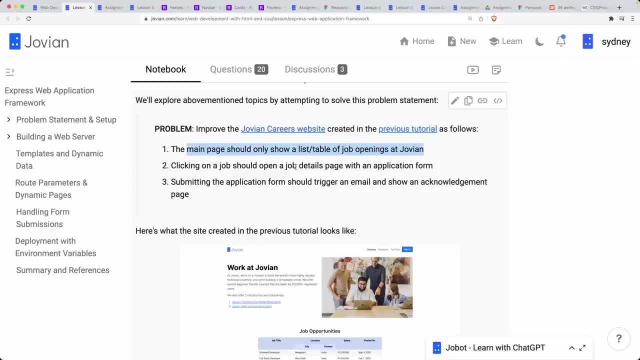 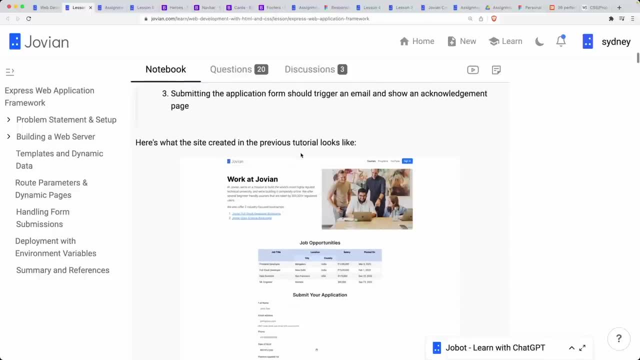 So we wanted to improve the job in careers website. This time we w. we wanted to have a single uh just only show the table, only show the jobs on the main page and then show the application form on individual job pages. And then we wanted to have uh, an application form that can trigger an email. 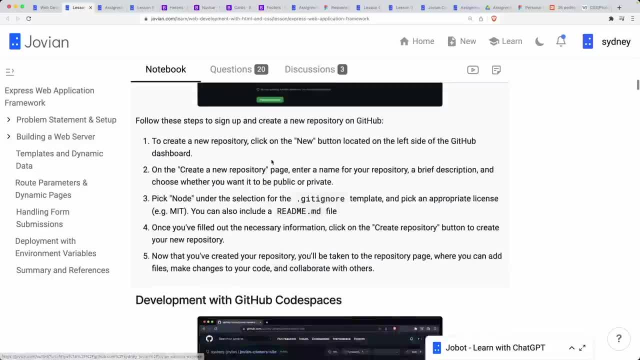 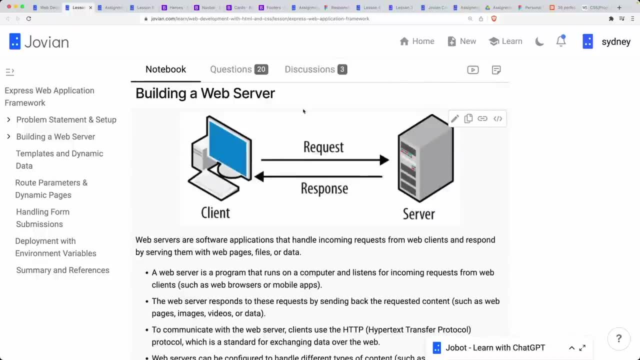 And an acknowledgement page. So this is what we did. Well, we we again created a new repository and we learned about creating web servers. So, instead of static websites where you simply open a URL and you get back in HTML CSS page of web server, can take a request and then do some processing. 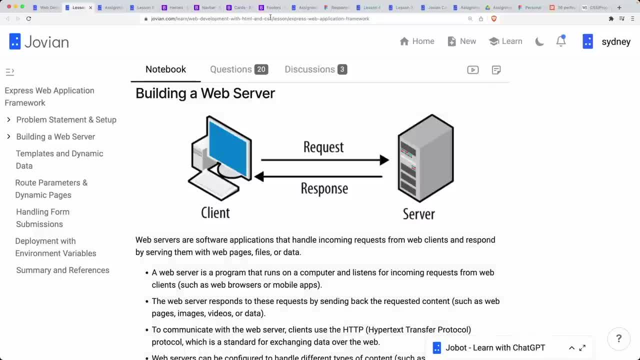 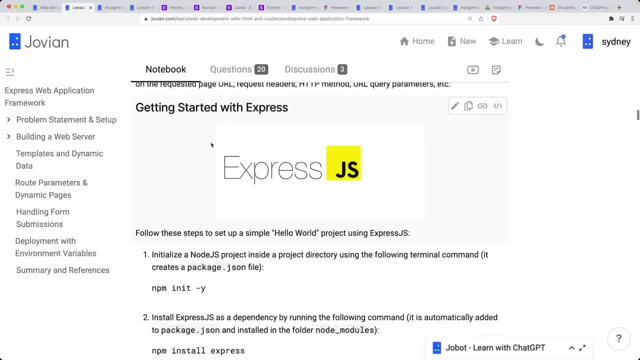 Maybe call a database or something, get some data from a database, like joviancom is doing, and then send it back. So we learned how to build web servers or web web applications And the way we did that is well. we use the express web application framework. So we learned how to build web servers or web web applications, And the way we did that is well. we use the express web application framework And we did this, and we have also seen a lot of the tools that we need to use to to do this as well. 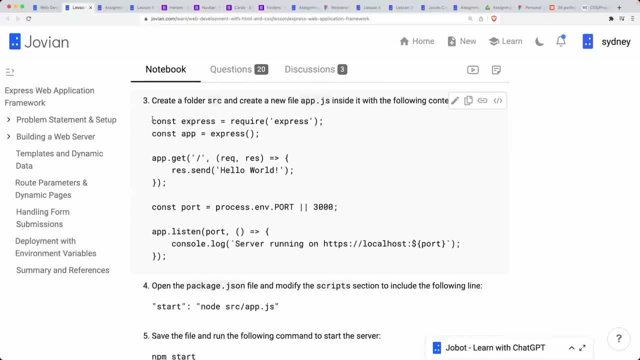 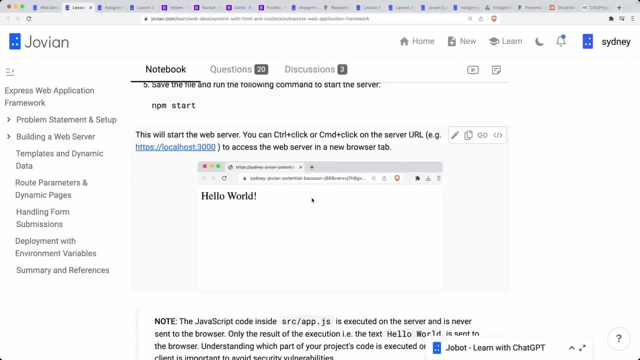 And we also did this to get back to the main page, for example, to the end of pages, which is really simple to get started with. you just create a bit of text like this, And you just write a bit of text like this And, as, just like that, you will get this when you open. 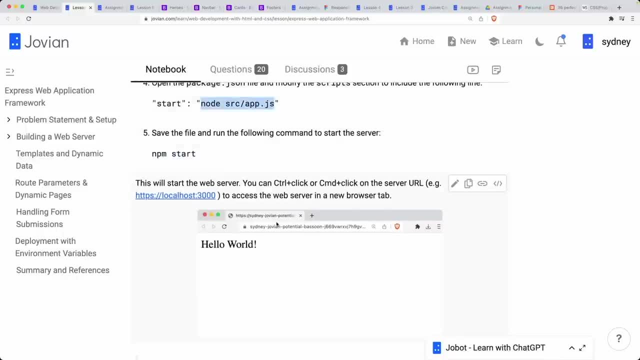 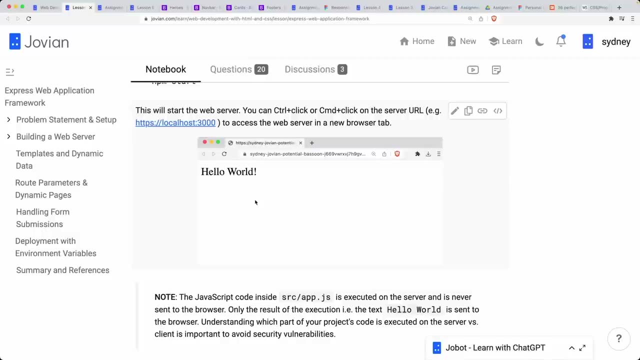 it up. when you run it using npm, start or node src appjs, you're going to get this hello world response And now you can start sending whatever content you want after doing whatever processing you need to do right. So the key benefit of web, of server side frameworks, is that you can do some 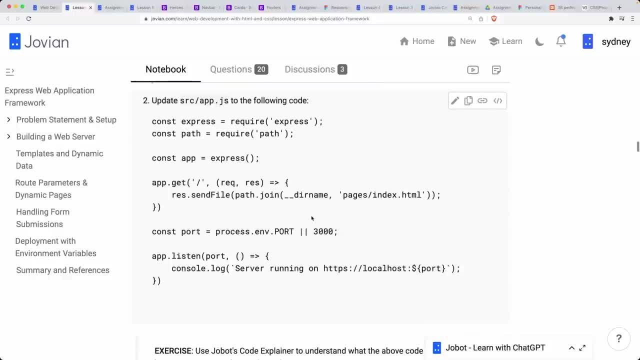 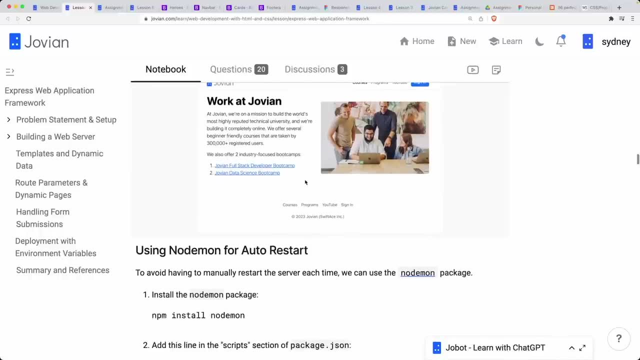 processing. So we saw how to serve HTML files. you can always just do rest or send file and send out a file like indexhtml, And this is what it looked like. Now, as we make changes, we don't want to keep restarting server again and again. that that's where you can use a tool like node mod. 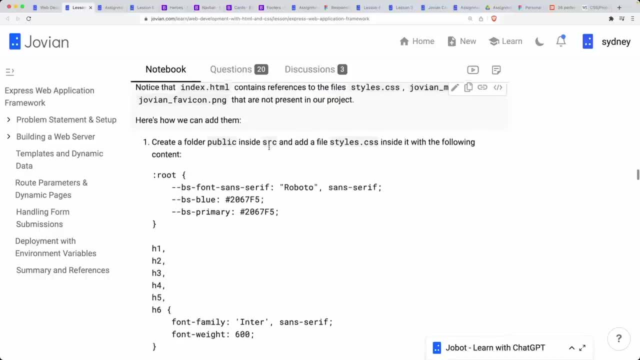 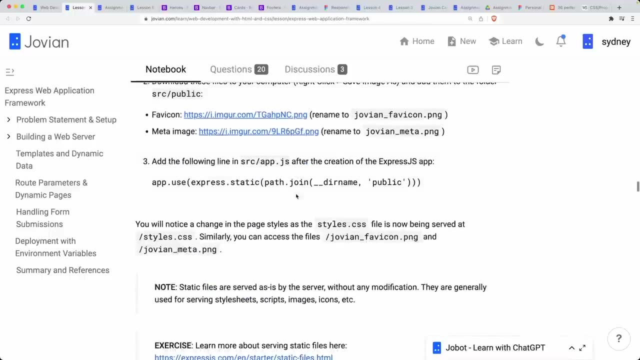 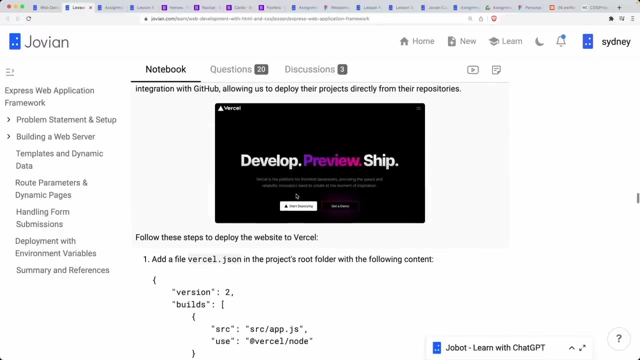 to automatically restart things. Then to serve static files, you can use express dot- use So express. or app dot- use express dot static. So any images, any CSS files are often served as static files, And deploying Express applications to Vercel is also fairly straightforward. you just is also fairly. 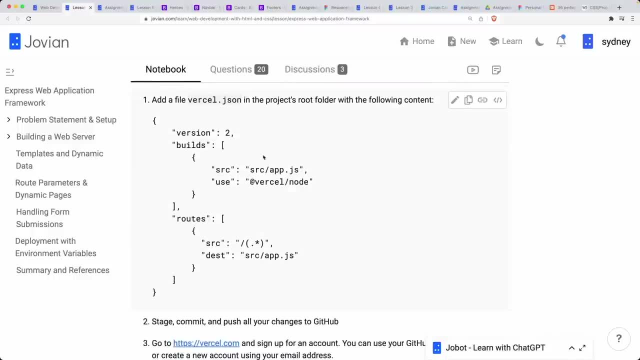 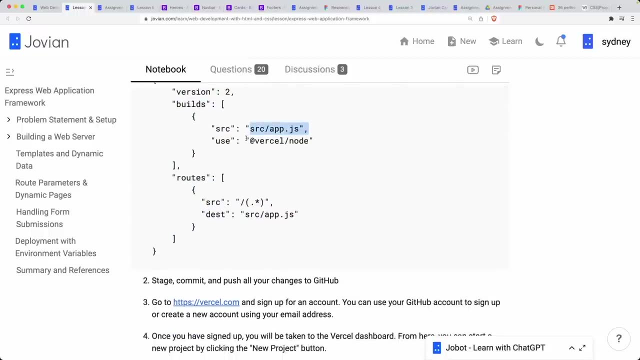 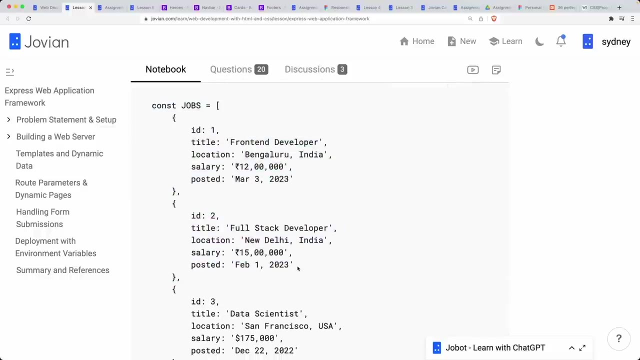 straightforward. you just need this Vercel dot JSON file in the projects root folder with some content that informs Vercel where to send all the requests and what environment to use. Okay now, next we looked at how to use templates. So let's say we had this list of jobs that came from a 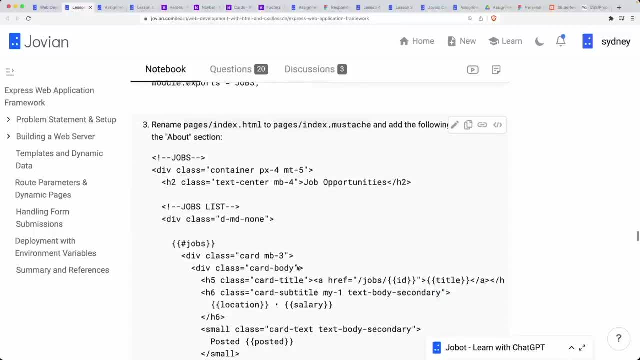 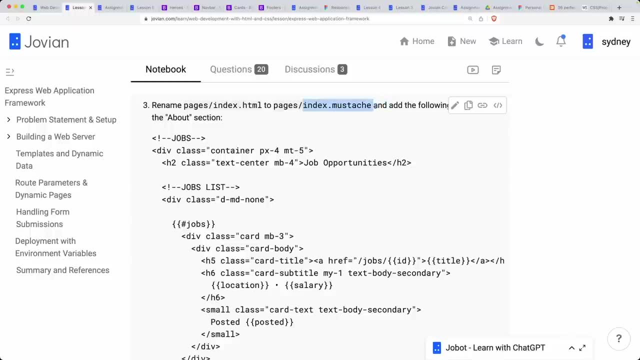 database, or maybe it's just something that we have hardcoded. Now we want to actually render it using a template, And that's where we can create a template. we can change indexhtml to index dot mustache And then inside it we can create this mustache template which can loop over. 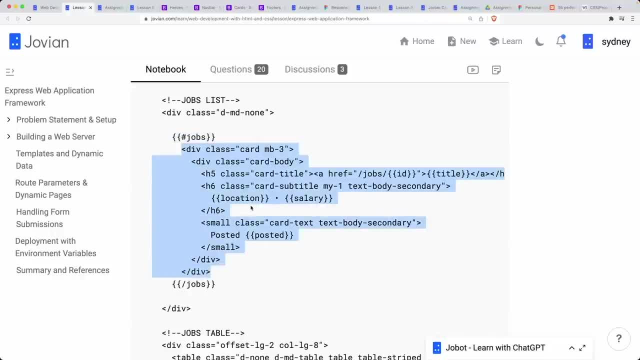 the variable jobs and then create a list of these cards And in each card insert the title, job title, job link and the salary and the posted date, And then, similarly, we can also create a table Once again that can loop over the list of jobs and create table rows. 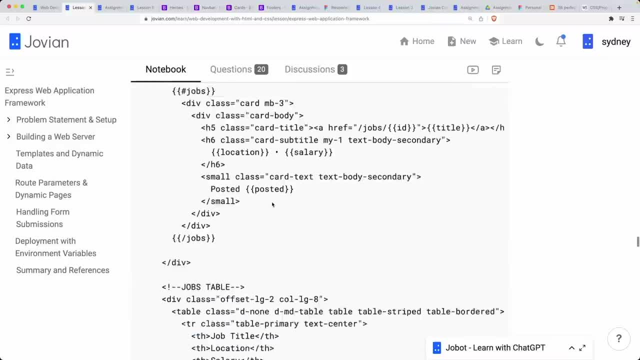 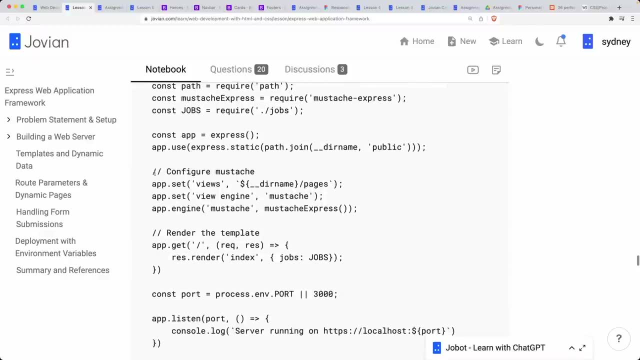 And the table will be shown on on desktop and on mobile will show the list of cards. So we are using code, HTML code, but this time we're putting it inside a template And we configure mustache as the view engine And then we simply render that index template. 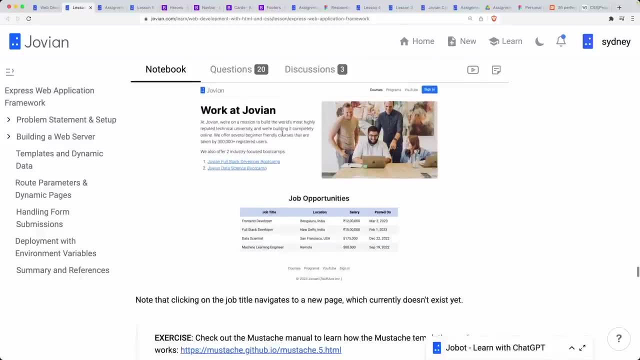 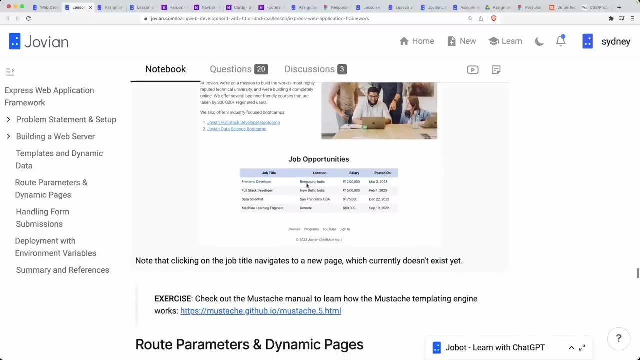 And we give it the data jobs, the list of jobs as the variable jobs And just like that. that renders this page or that renders this table on mobile on desktop and a list of cards on mobile And there are a bunch of things you can do with mustache. it's really easy to use. 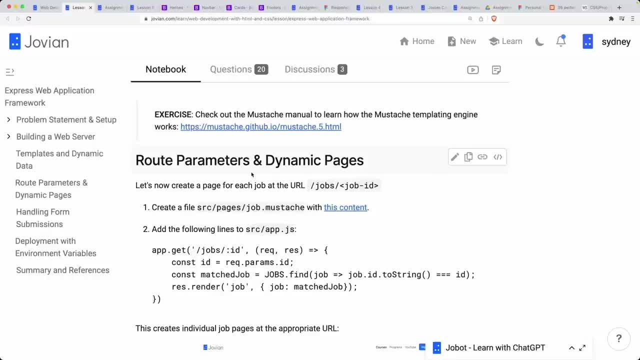 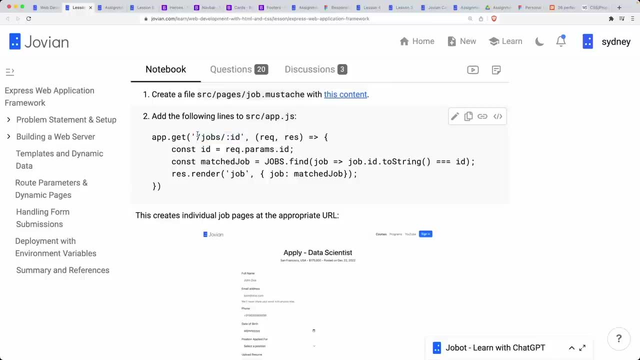 But the idea here is you take some data and you put it into some HTML, you put it into a template to render a page. then we also looked at route parameters. So if you have a route like this: app, dot, get slash jobs, colon ID, then you can take your, you can take some logic and 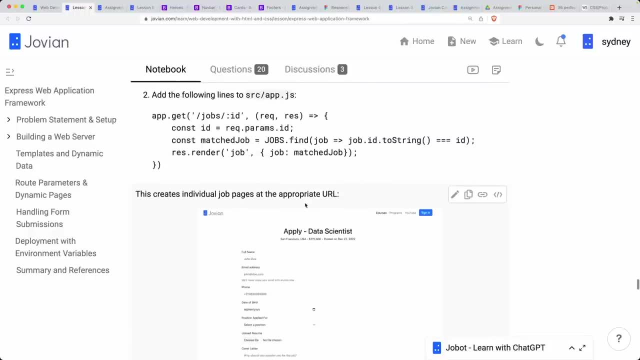 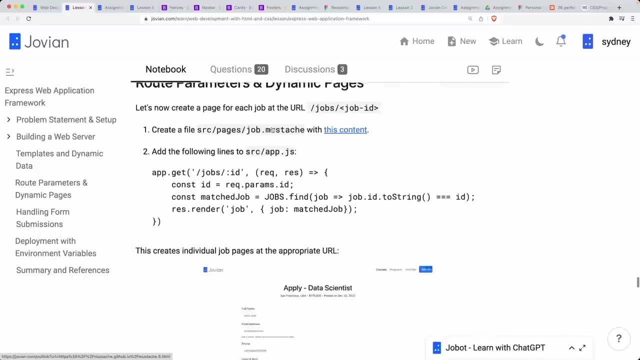 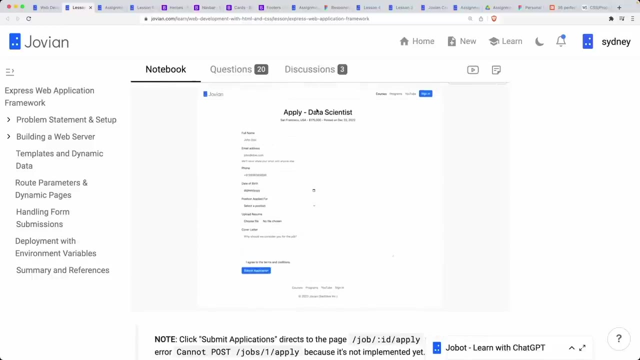 then use that to render different kinds of dynamic pages. For example, here we have this template called Yeah, we had. we have a template called job. So we have a template called job And in that template, job dot mustache- we take the application form and we render the title of the job right, And that's what that. 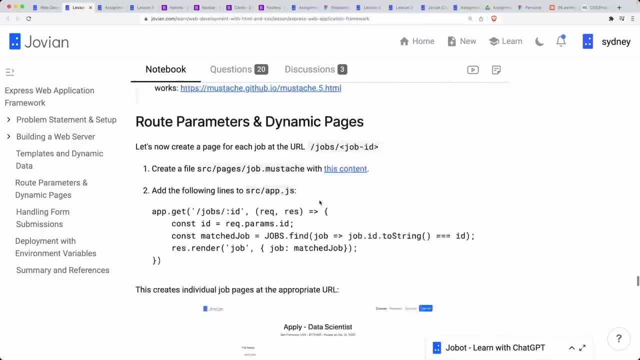 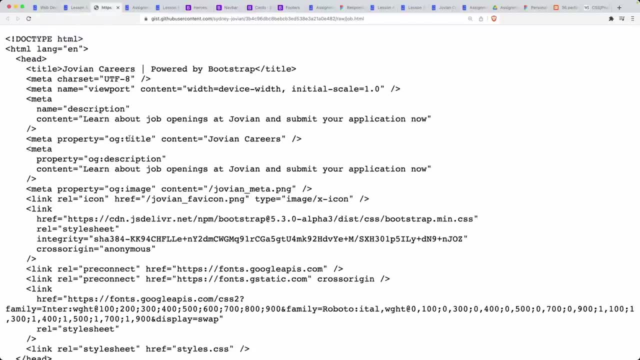 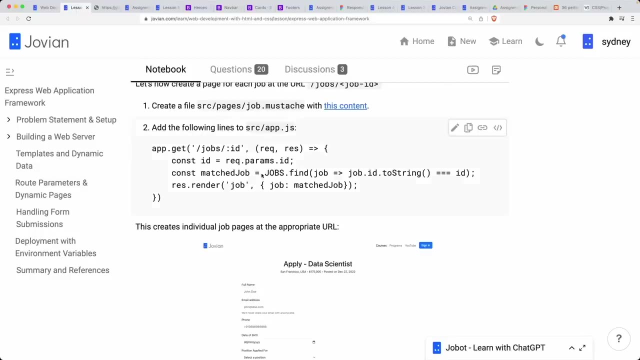 looks like I believe the job template is: Yeah, some, it's a, you all the source code. Yeah, here is the template content for the job template, right? So it contains just: it's going to use the job title And it's going to show that job title in here. it's in the application form at: 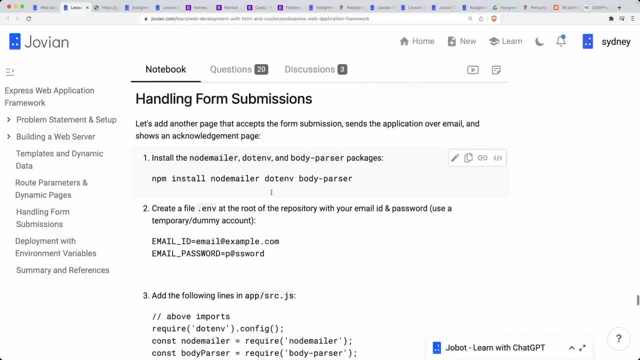 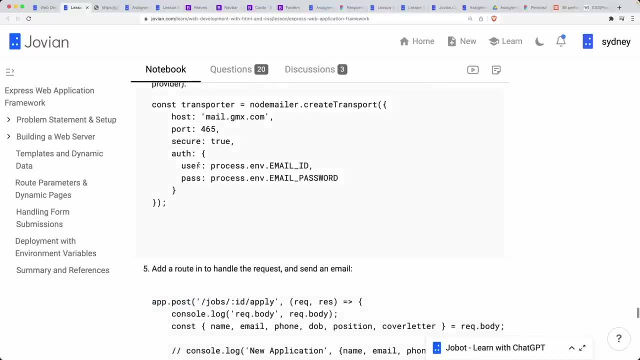 the title of the application form. All right. Then we looked at how to handle form submissions. Now, to handle form submissions, we need to use this app- dot post route Okay- and we need to also give it when you also need to use. 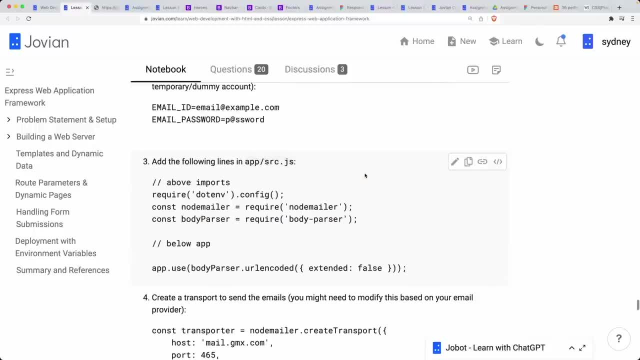 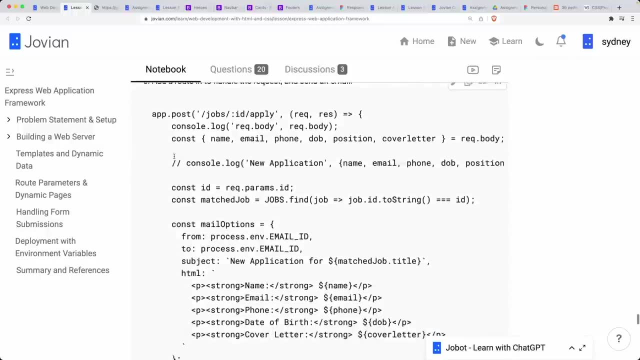 this body parser middleware so that it can pass the content that is going to be sent using the post method And, finally, we can store the form responses in a database. But what we chose to do instead was to simply format an email and send it. send out an email using the node mailer package. 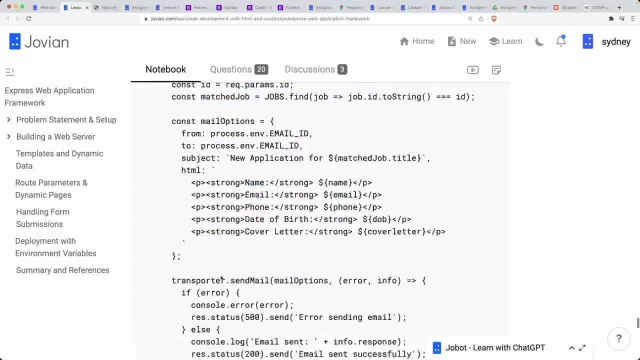 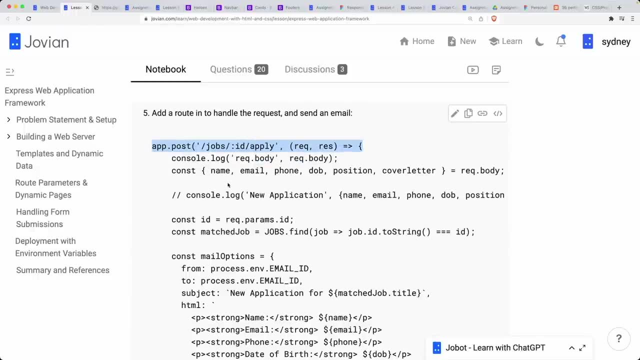 Okay, so the idea is not that every form response has to be emailed, But you can get that form response into a route And then you can do whatever you want to do with it. So let's go ahead and do whatever you want with it. store it in a database, just throw it away, send out an email.